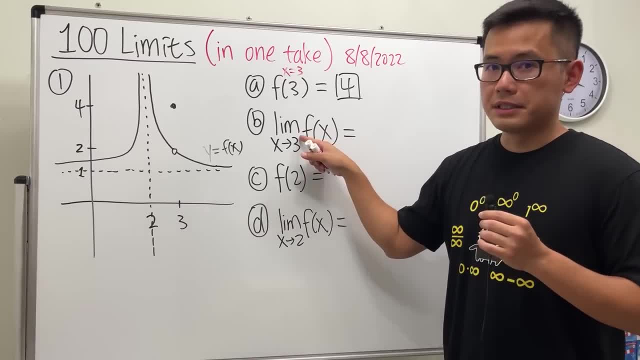 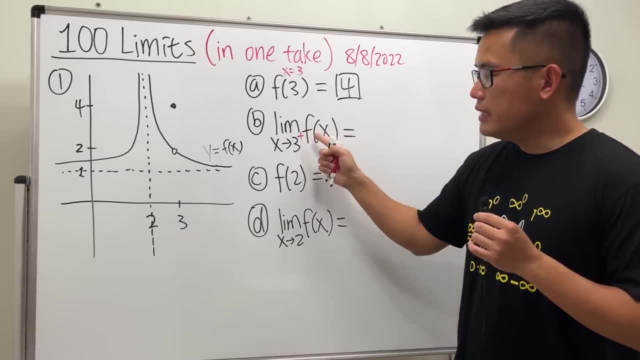 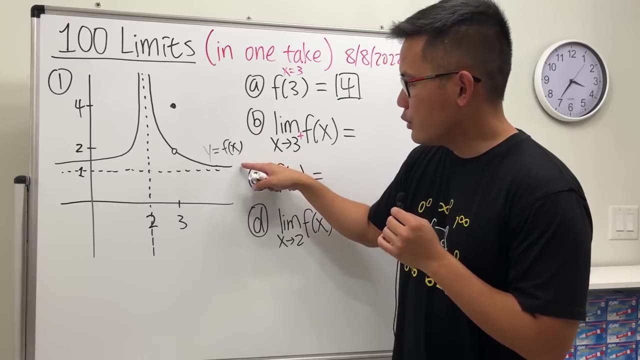 So here's the deal. You see how we do not have the plus or minus here. We actually have to do both. So look at when we have the positive version right here. This means we are approaching the 3, right, when x is 3, from the right, So you can use your right hand and then you 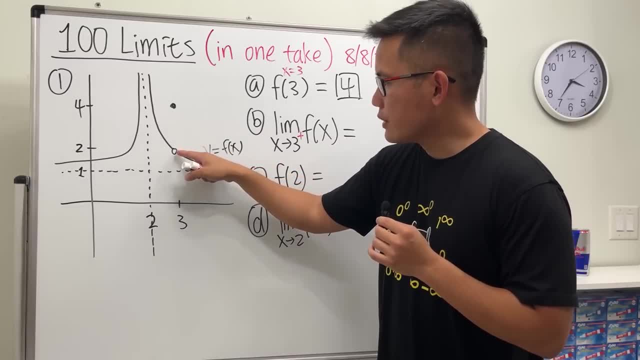 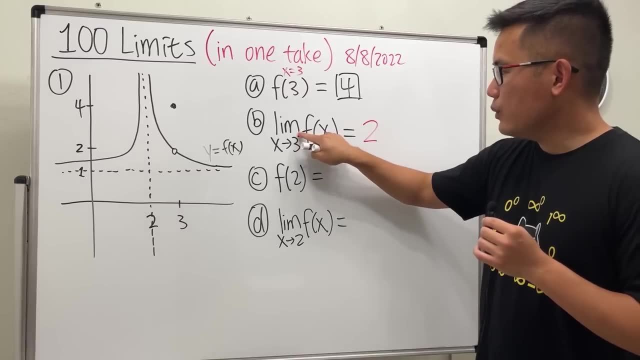 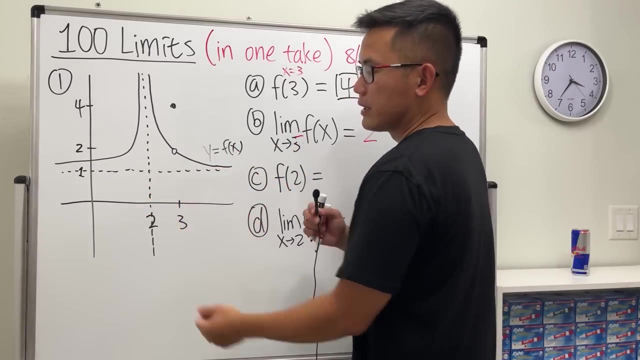 are approaching and look at the y value and you see the y value is approaching 2.. So when x is approaching 3 plus, we get 2.. So keep that in mind And then we also have do the minus, meaning that you can use your left hand because we're approaching three from the 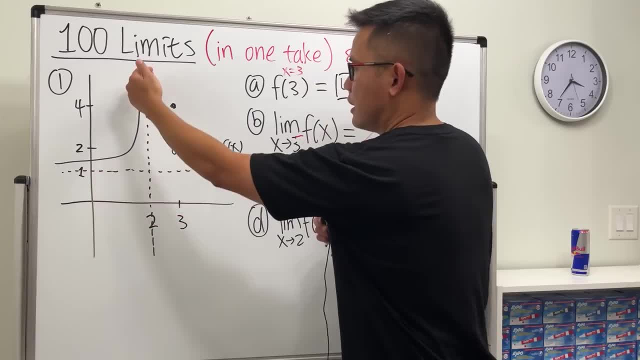 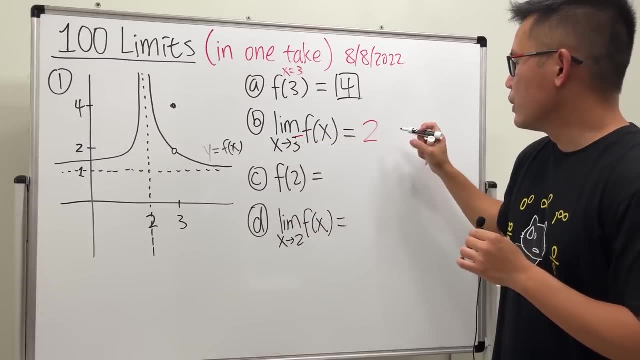 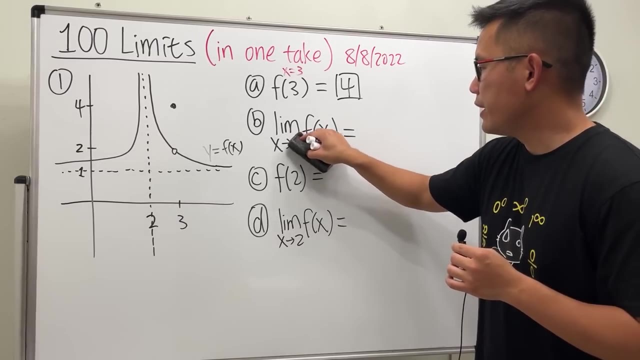 left hand side, so you can start here, because it's approaching here. and you see, it's like this, and the y value is also approaching two. so when x is approaching three minus, we also get two, and two and two are the same. so the answer for this right here, when there is no plus or minus. well, 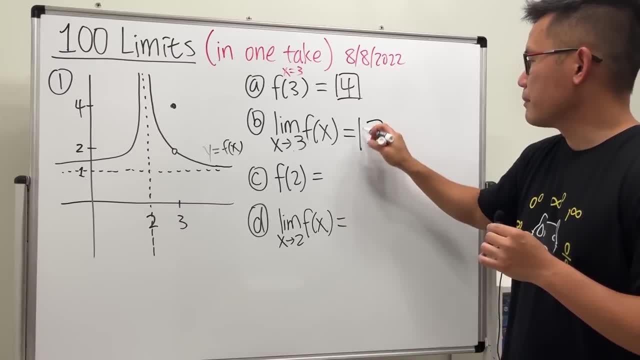 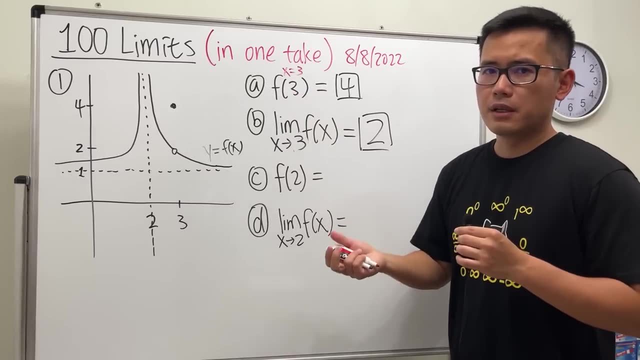 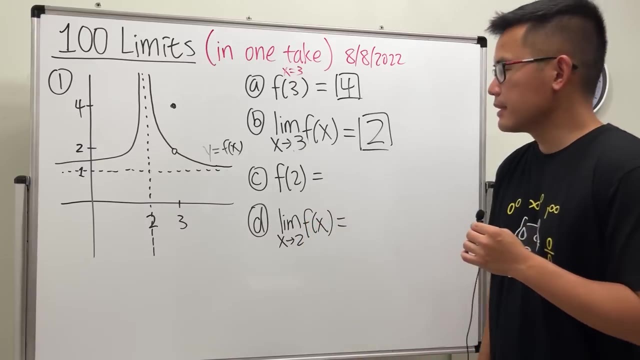 the answer is just equal to two right. keep that in mind and you see how these two questions are very different. this is the typical. look at the graph, look at the closed circle question and this right here you really have to start to worry about the calculus part of the limits. all right, now let's 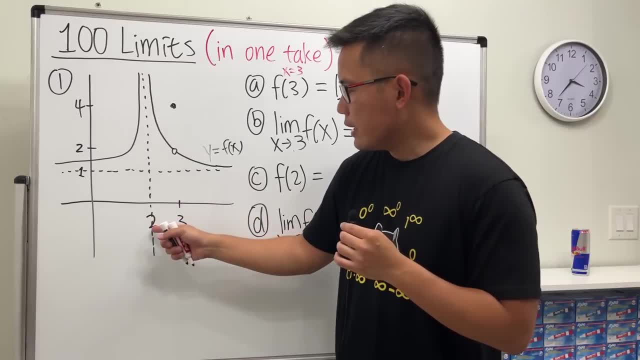 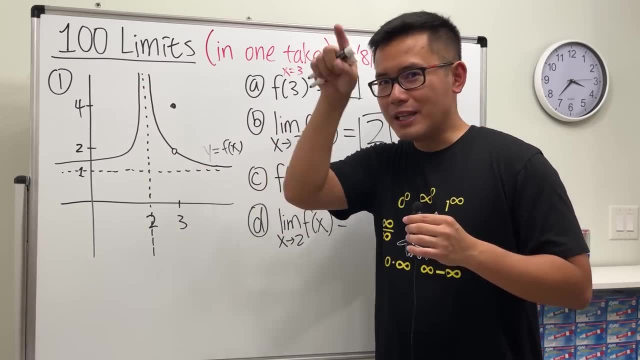 see f of two. f of two we go to x is equal to two. uh, that's the vertical acetone, like this, no dot. well, technically, the reason i put down of cut is just because of the vertical acetone. but yeah, we do not have the value of the function. 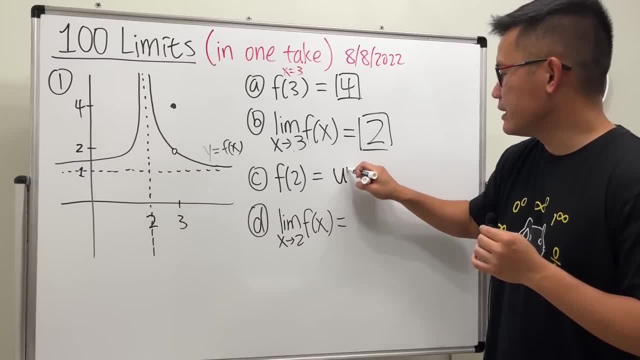 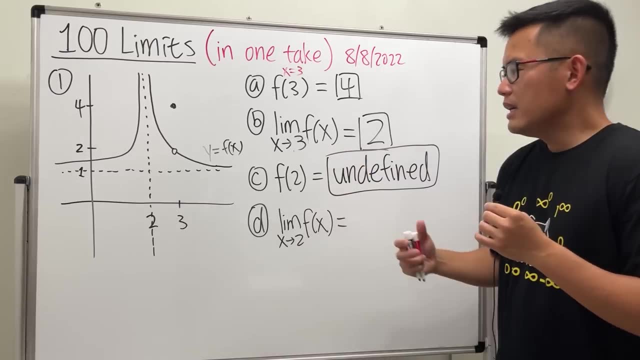 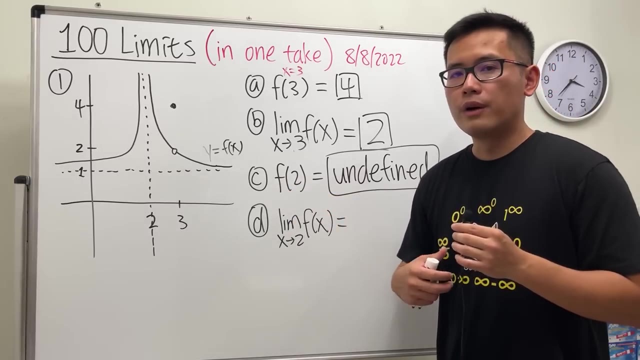 over there. so in this case what we say is undefined, and there is a small difference between undefined versus does not exist. both of them kind of mean that we do not have the answer. but undefined is when we are talking about the value of a function or computation. so 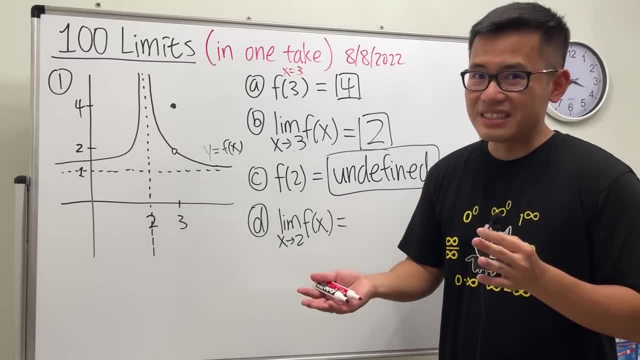 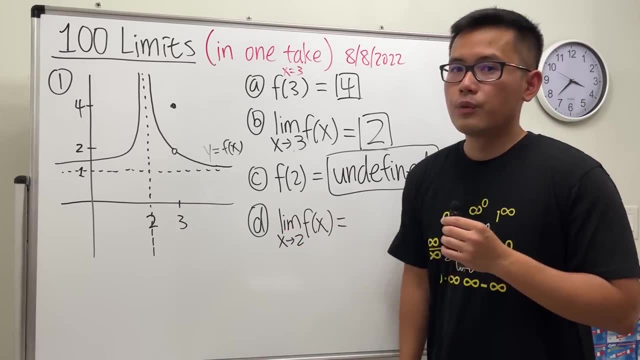 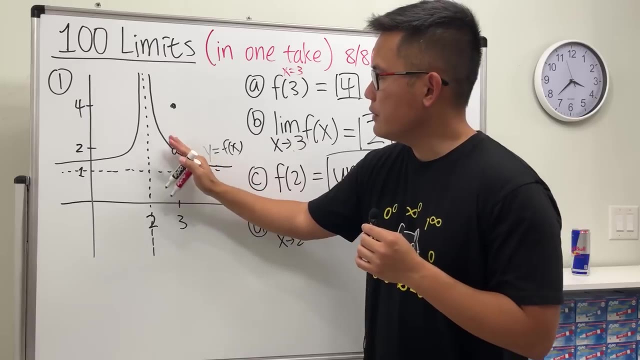 just keep that in mind. if the limit doesn't have the answer, then we say the limit doesn't exist. all right here. lastly, we have the limit as x approaching two. well, again, we do not have the plus or minus. we check both. if we go to the two from the right, you see that the curve is. 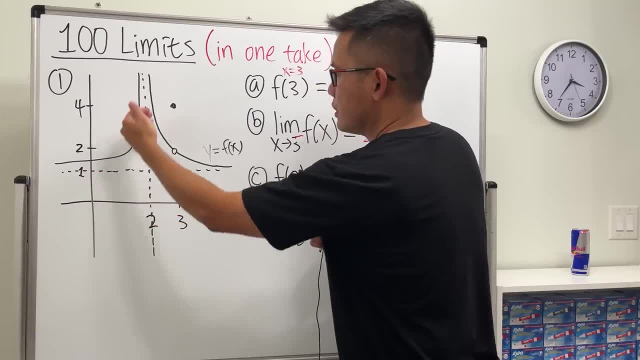 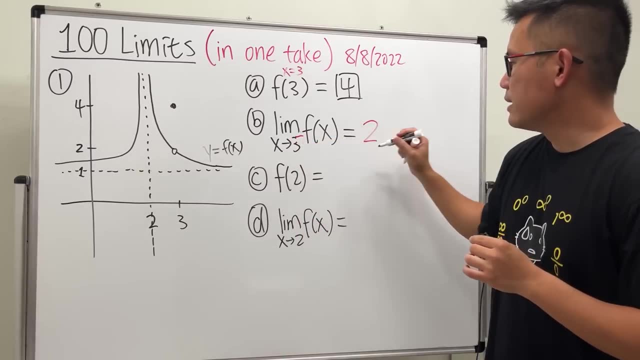 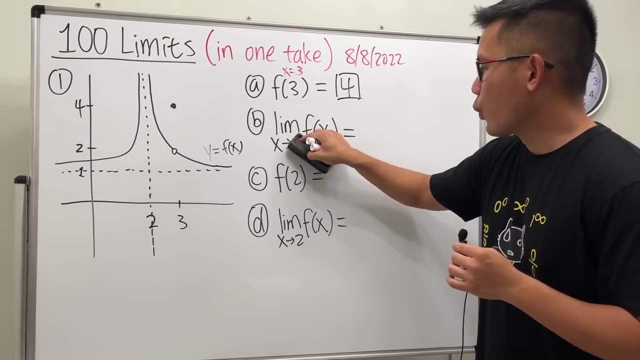 from the left hand side, so you can start here, because it's approaching here. and you see it's like this: and the y value is also approaching two. so when x is approaching three minus, we also get two, and two and two are the same. so the answer for this, right here, when there is no plus or minus, 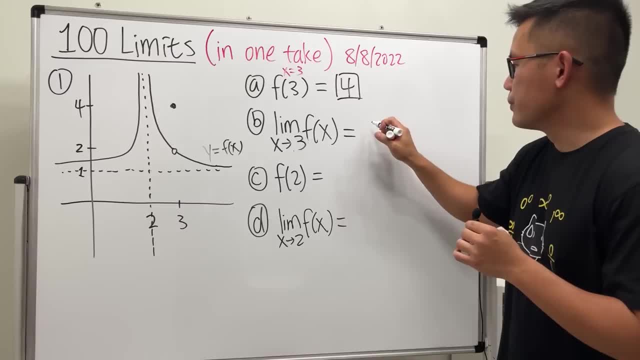 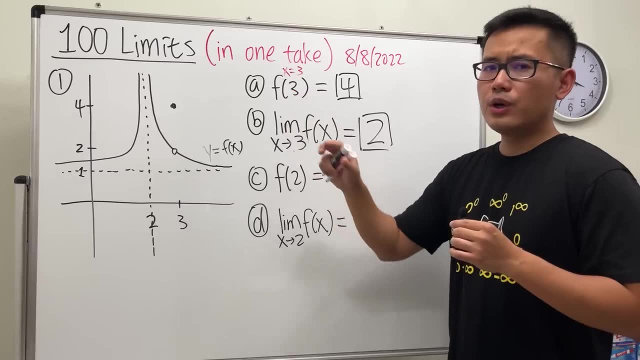 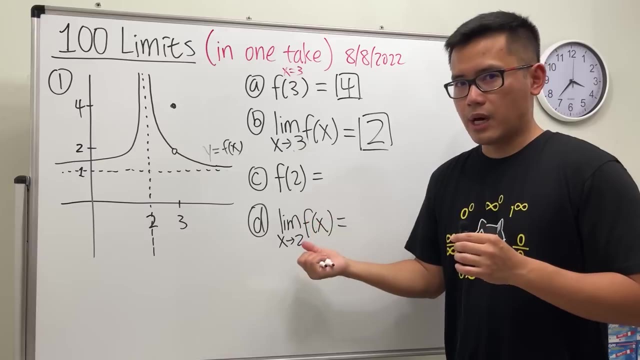 well, the answer is just equal to two right. keep that in mind and you see how these two questions are very different. this is the typical. look at the graph, look at the closed circle question and this right here you really have to start to worry about the calculus part of the limits. 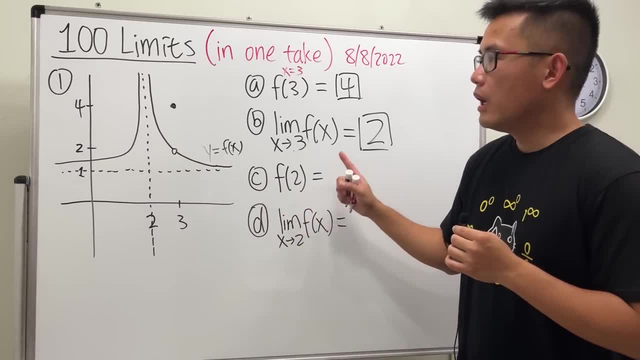 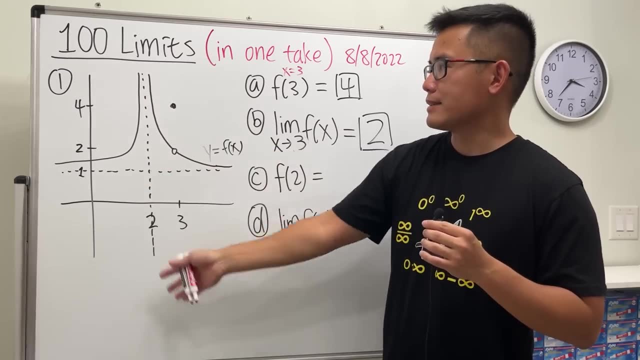 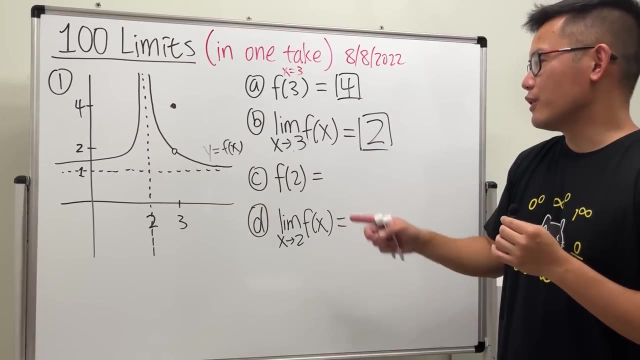 all right. now let's see f of two. f of two we go to. x is equal to two. uh, that's the vertical acetone. like this, no dot, what's that? technically, the reason I put tons of cut is just because of the vertical isotope. but yeah, we do not have the value of the function over there. so in this case, what? 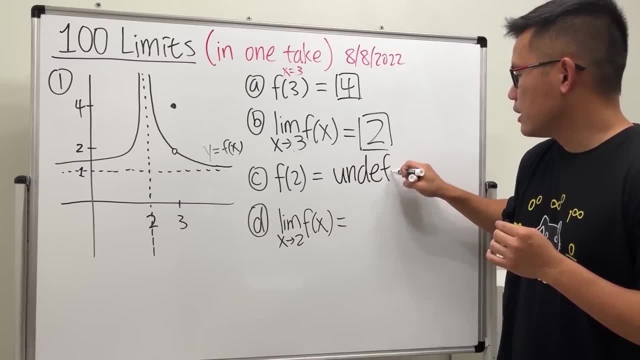 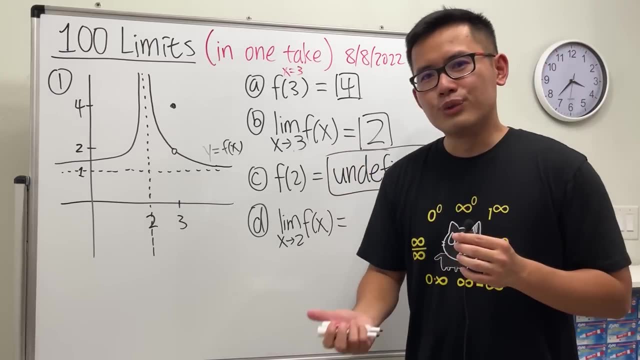 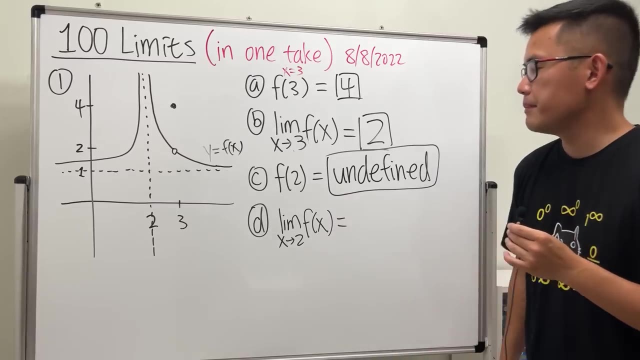 we say is undefined, and there's a small difference between undefined versus does not exist. both of them kind of mean that we do not have the answer, but undefined is when we are talking about the value of a function or computation. so just keep that in mind. if the limit doesn't have the answer, then we say the. 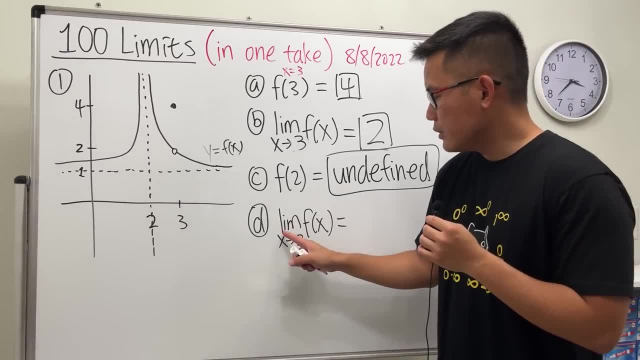 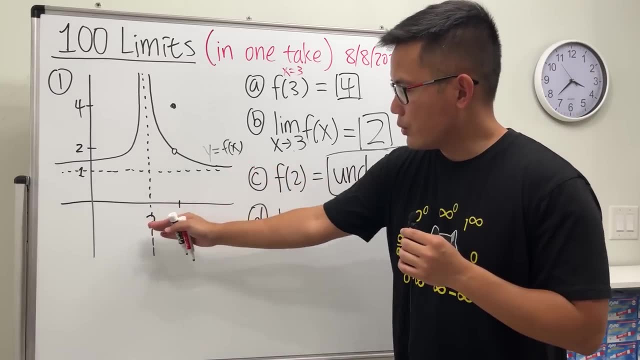 limit does exist. all right here. lastly, we have the limit as X approaching 2. well, again, we do not have the plus or minus, we check both. if we go to the 2 from the right, you see that the curve is going straight up. so that's positive. 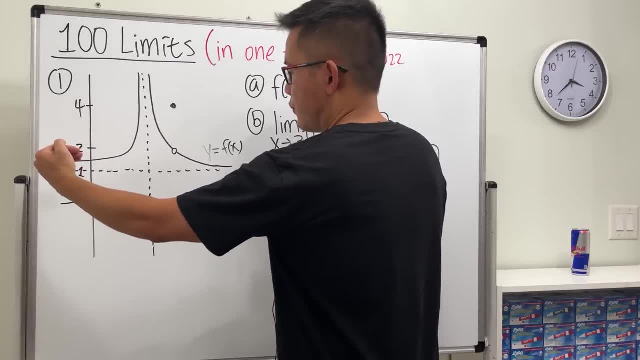 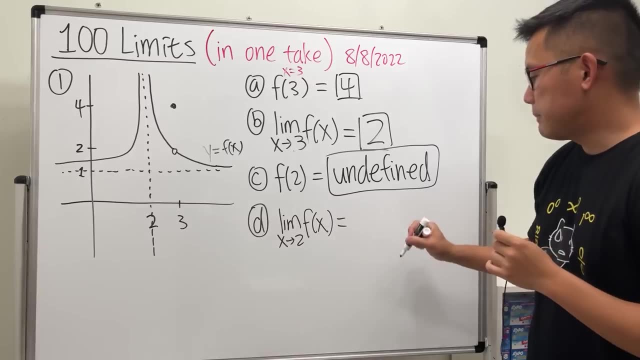 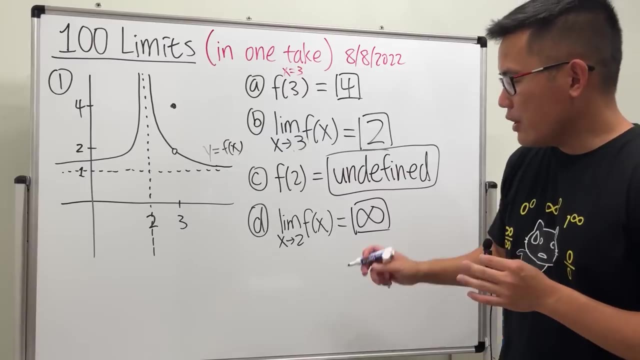 infinity. and if we approach 2 from the left hand side, you see the curve. it's also going straight up. so both are going straight up, meaning positive infinity. so be sure you check both. all right, so that's pretty much it. however, let me just give you guys two more like a extra. 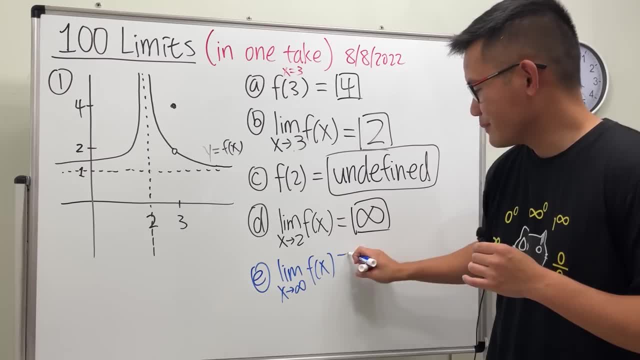 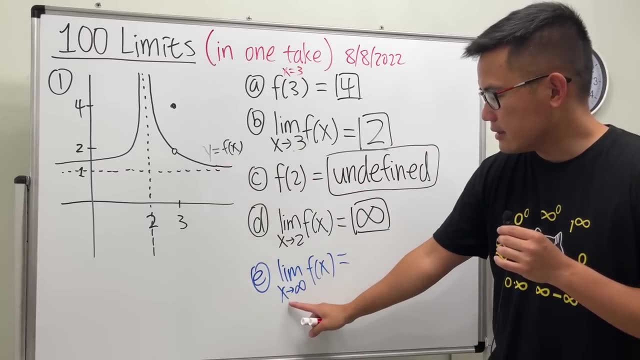 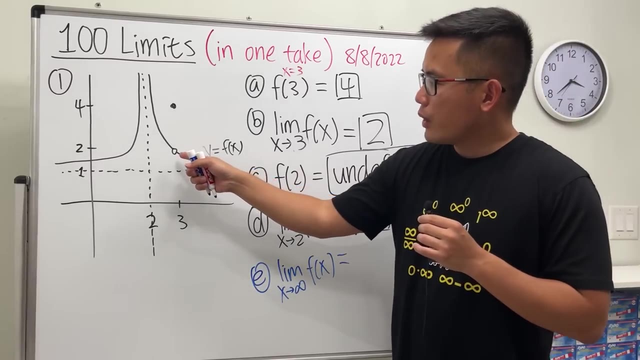 practice- yeah, this is not on the file to make you guys feel special, because we have the horizontal isotope as well, and that's the case when X is approaching positive infinity. this means X is all the way to the right, and when you have the picture right here, you see how it's impossible for us to include everything. 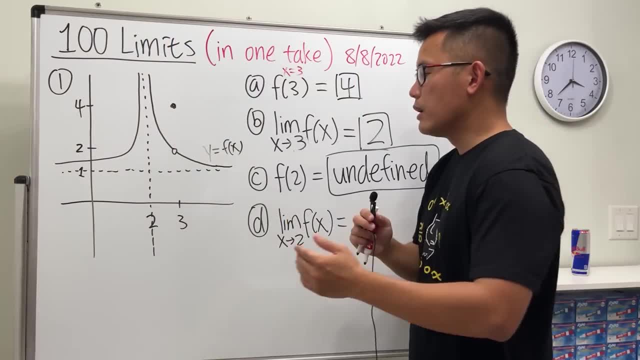 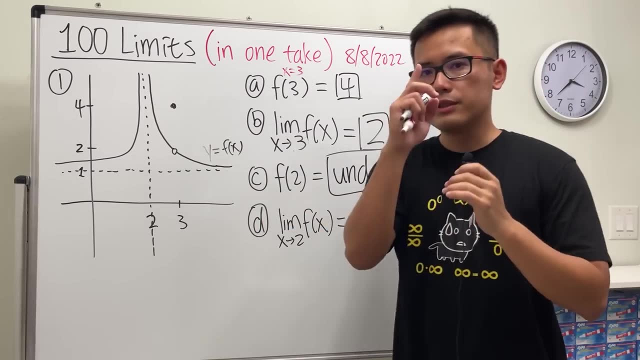 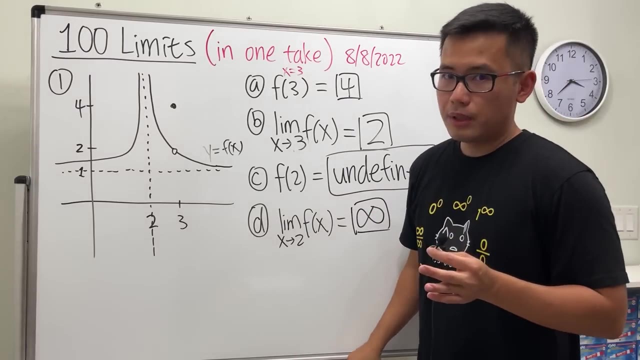 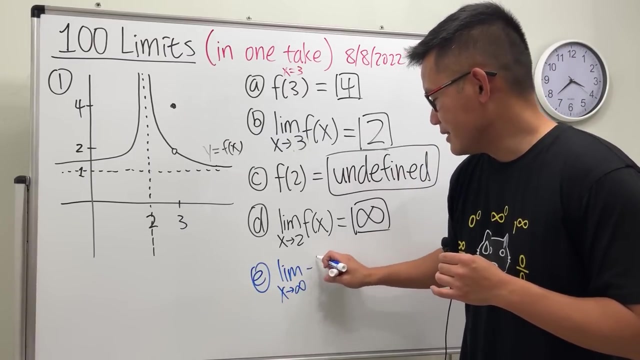 going straight up, so that's positive infinity. and if we approach two from the left hand side, you see the curve is also going straight up, so both are going straight up, meaning positive infinity. so be sure we check both, all right. so that's pretty much it. however, let me just give you guys two more like a extra practice. yeah, this is not on the file. 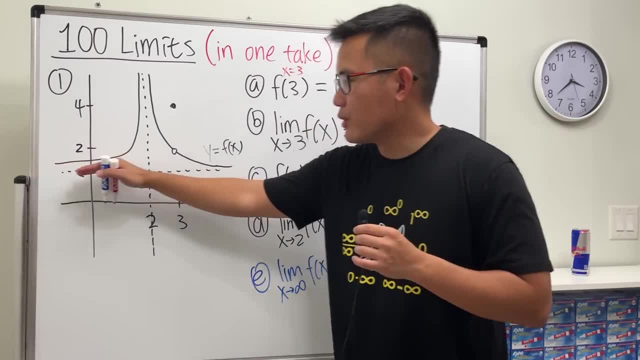 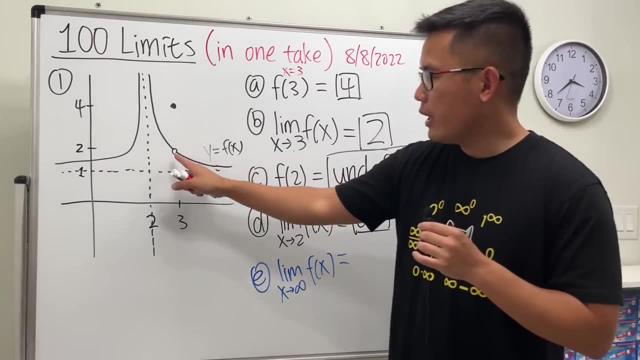 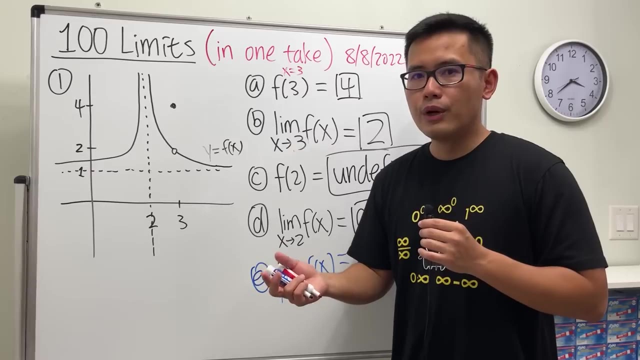 to make you guys feel special, because we have the horizontal as the best will, and that's the case when x is approaching past infinity. this means x is all the way to the right, and when you have the picture right here, you see how it's impossible for us to include everything. 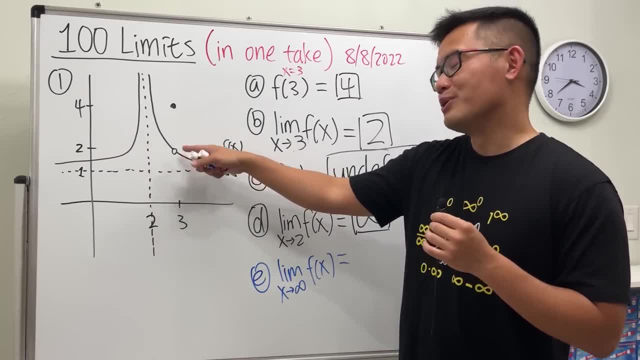 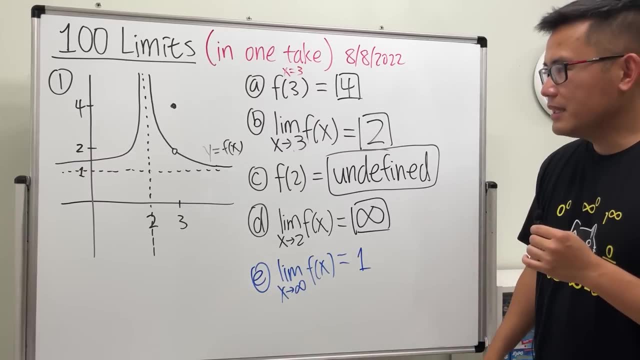 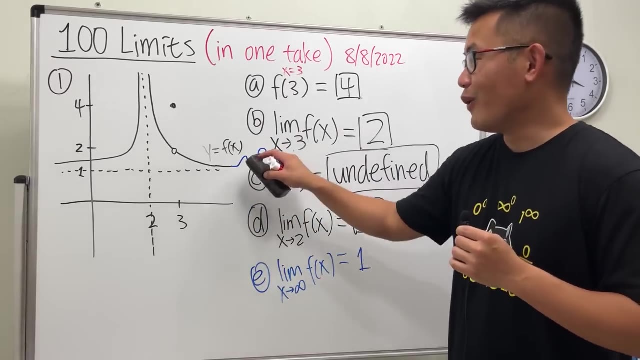 so you just have to kind of just assume that, okay, it's just going to follow this pattern. the y-foil is going to approaching one, all right, so you're not going to see like this and then, oh no, no, nobody will do that to you. hopefully that's not the case, especially on the test. if you are. 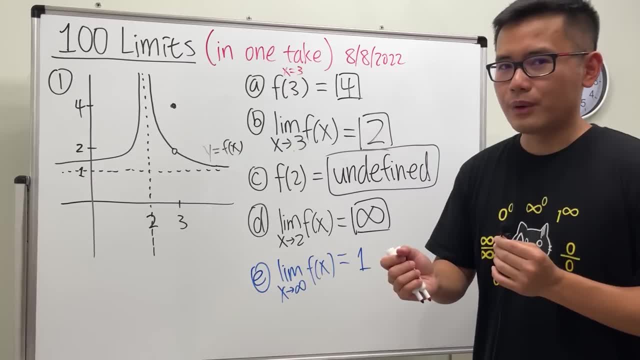 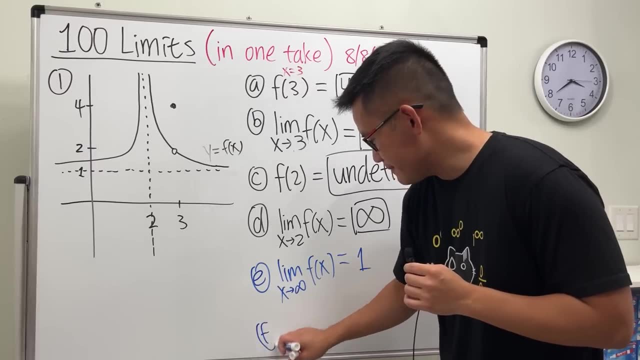 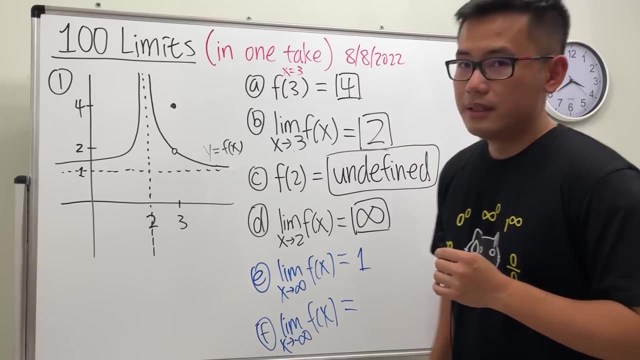 given a graph, nobody will do that to you. however, though, if you are using a graphing calculator, if you're grabbing like a weird function, maybe you have to worry about it. but yeah, that's a different story anyway, okay, limit as x approaching negative infinity. f of x, this case we are approaching left. 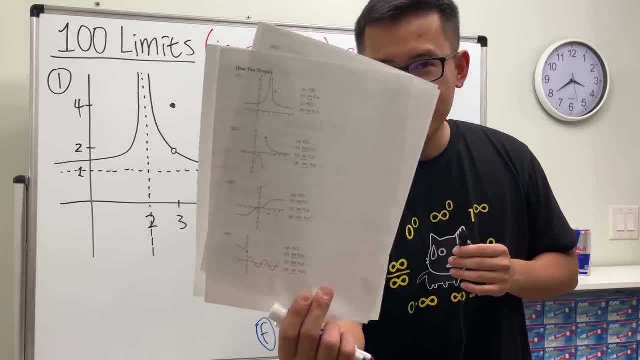 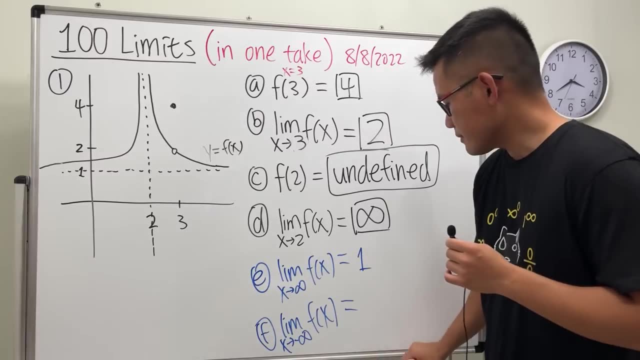 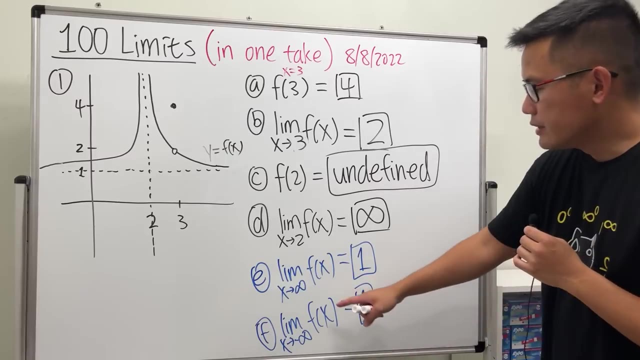 all right, and then if you look at a better picture from the file, it's actually approaching one as well. so this is more like this, it's more like that. yeah, so here are some terminologies that we just would like to go over. you'll see how, when x is approaching infinity, we get one. 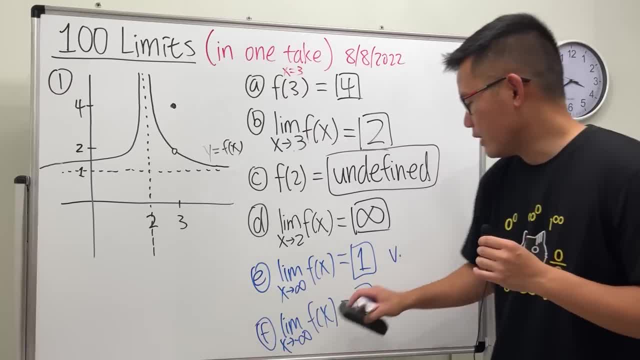 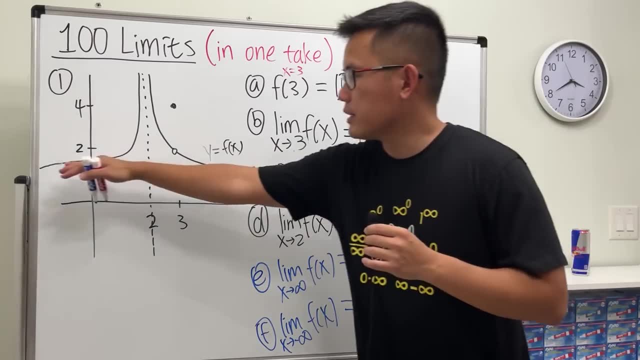 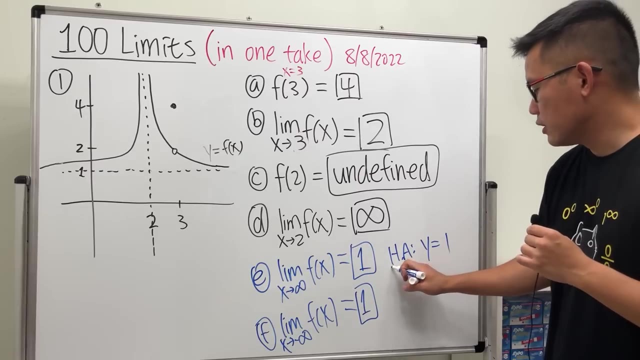 this means we have a vertical. so this means we have a horizontal acetone when y is equal to one. right, that's the horizontal dash line right here, and likewise we also have one, so you don't have to write down the one twice. so we have a horizontal acetone at y is equal to one, and you see how, when x is approaching to. 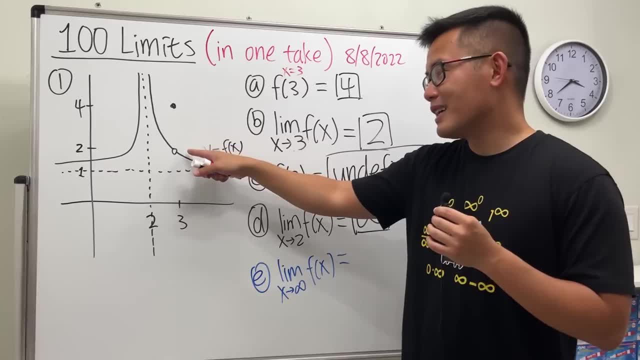 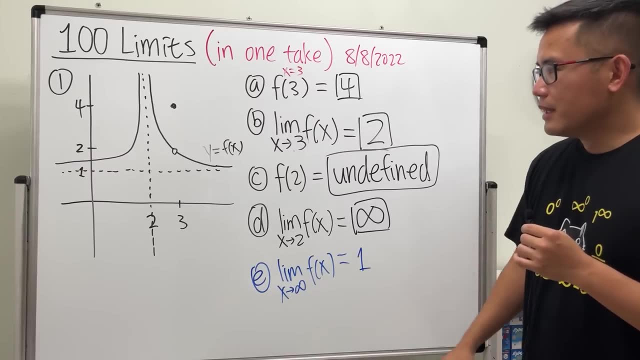 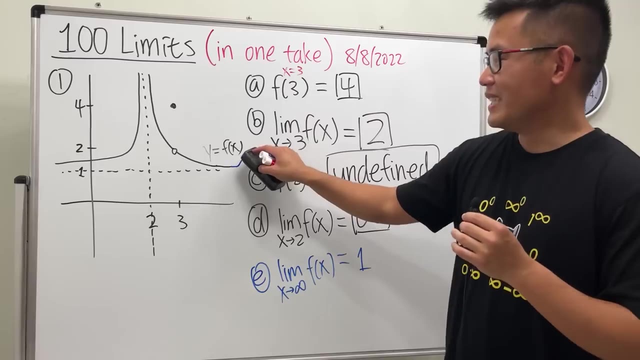 so you will just have to kind of just assume that, okay, it's just going to follow this pattern. the y-foil is going to approaching one, all right, so you're not going to see like this and then, oh no, no, nobody will do that to you, hopefully. 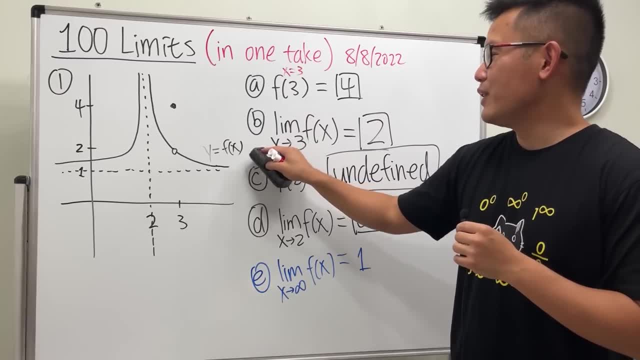 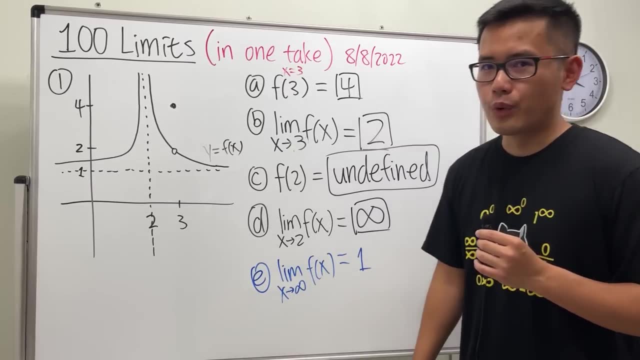 that's not the case, especially on the test. if you're given a graph, nobody will do that to you. however, though, if you're using a graphing calculator, if you're grabbing like a weird function, maybe you have to worry about it. but yeah, that's a different story. anyway, 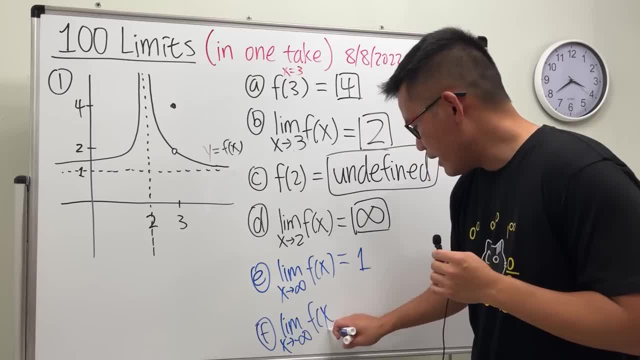 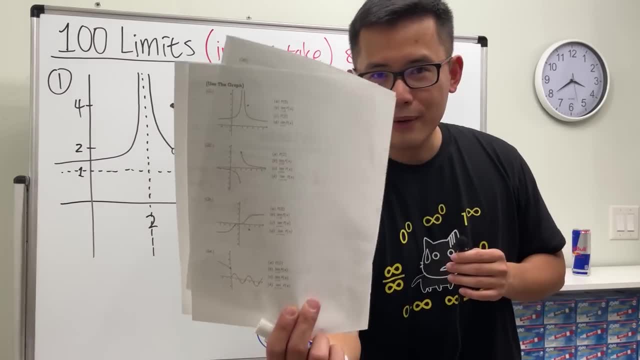 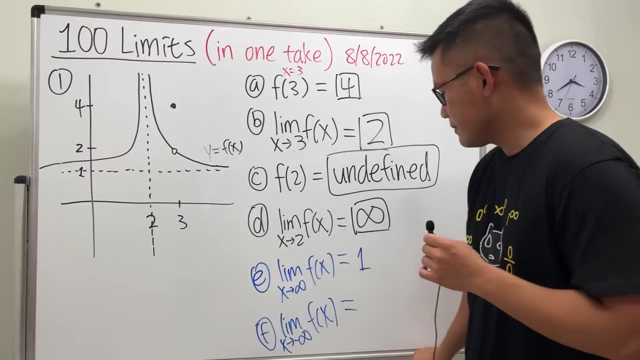 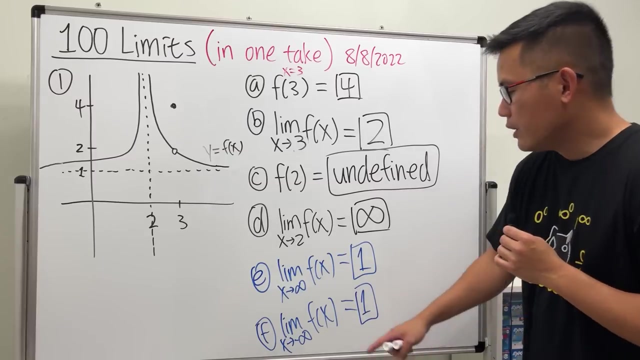 limit as X approaching negative infinity, f of X. this case we are approaching left, all right, and then if you look at a better picture from the file, it's actually approaching one as well. so this is more like this, it's more like that, yeah. so here are some terminologies that we'll also like to go over. you'll see how. 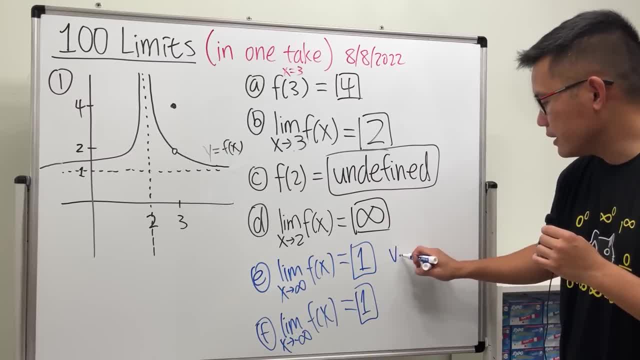 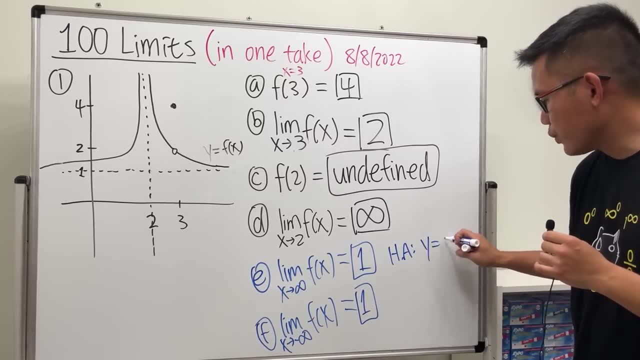 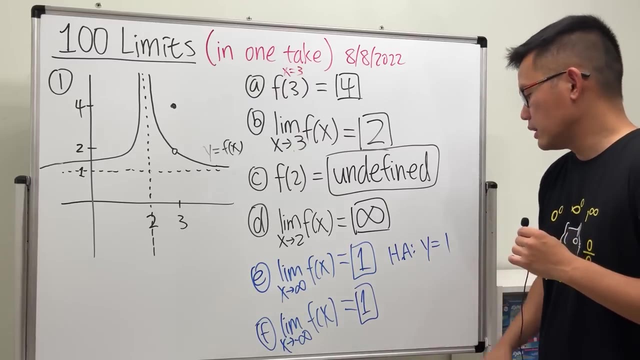 when X is approaching infinity, we get one. this means we have a vertical- sorry, this means we have a horizontal acetone. when y is equal to one, right, that's the horizontal dash line right here, and likewise we also have one, so you don't have to write on the one twice. so we have a horizontal acetone. 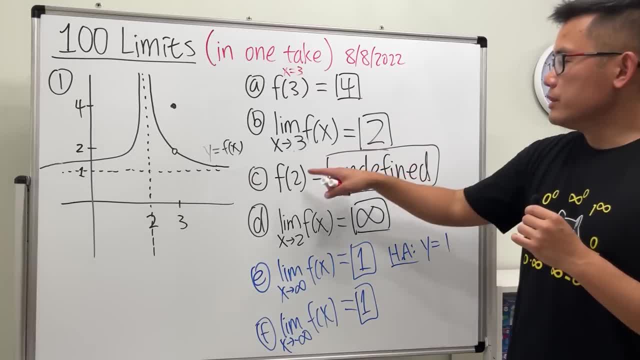 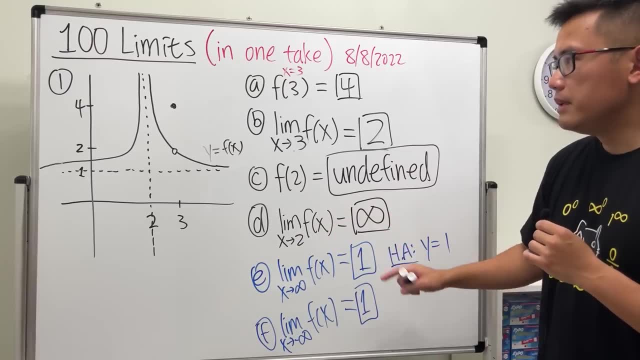 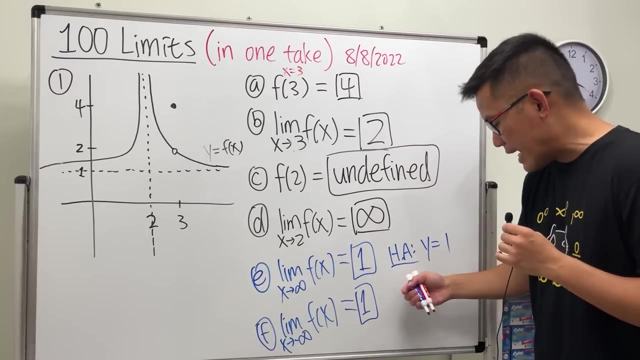 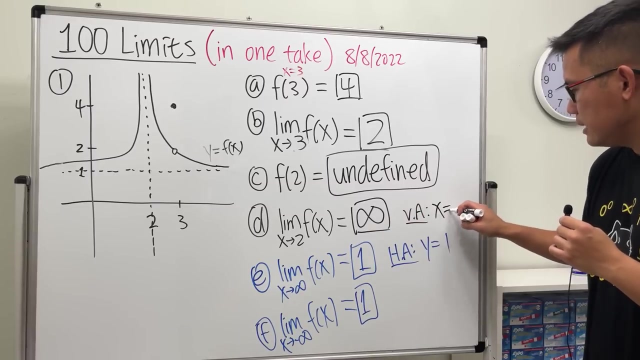 at y is equal to one, and you see how, when X is approaching two, the function, this limit, gives us Infinity. this means the function is going straight up. sometimes you may have a negative infinity, meaning go straight down. that's the case that we have vertical acetone, so vertical as well. at X equals 2, so that's the vertical dashed line. 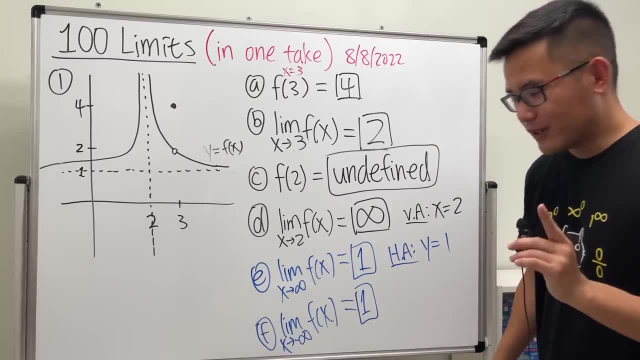 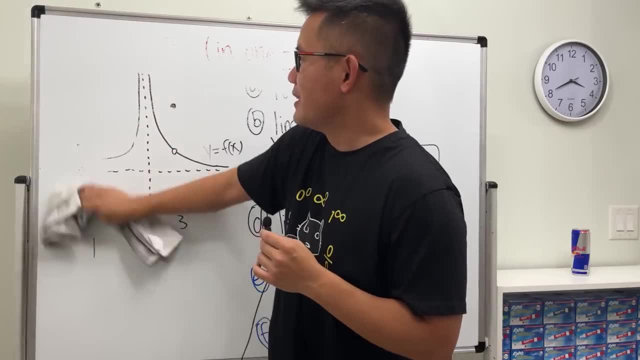 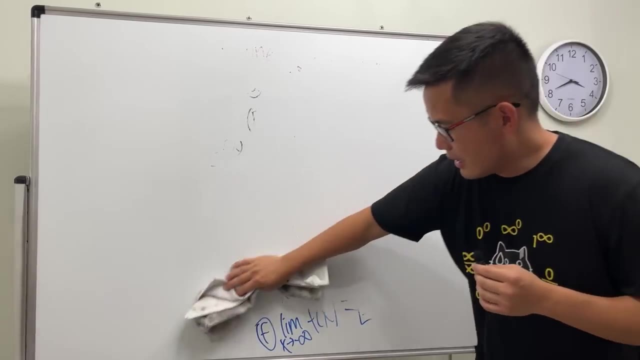 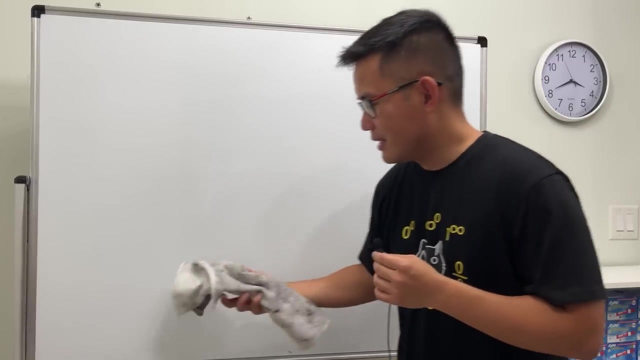 right over there. so there you have it. this is the first question and we have just a couple more to go, and yeah, so let me just erase this for the first couple questions. just maybe use the timestamp to navigate, especially because I will have to take some time to graph the function. so yeah, I'll try to I also. 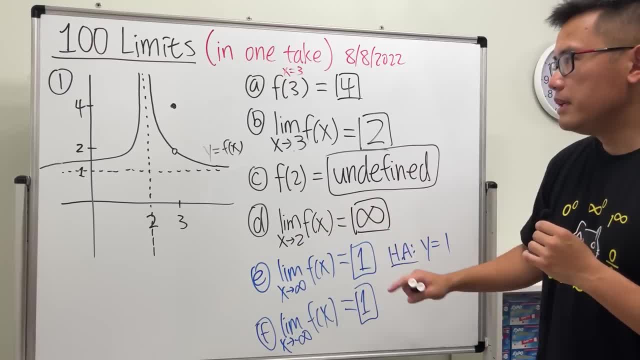 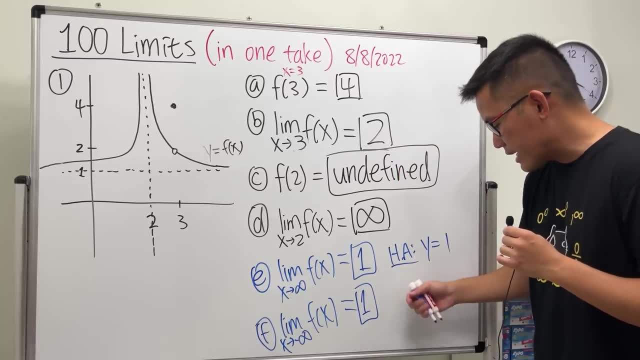 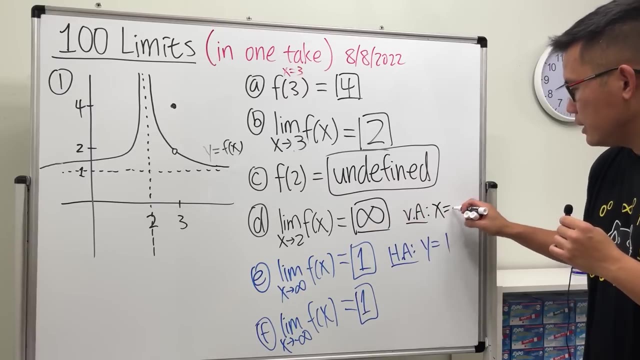 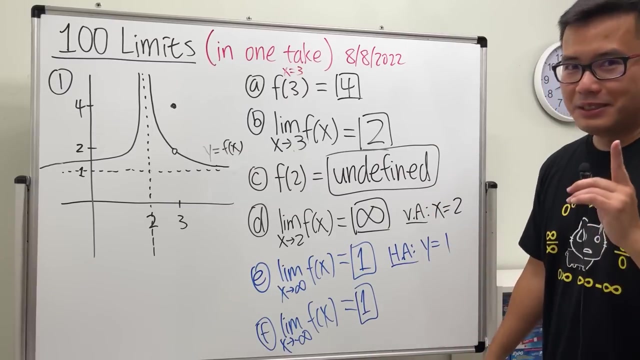 the function. this limit gives us infinity. this means the function is going straight up. sometimes you may have negative infinity, meaning go straight down. that's the case that we have vertical acetone, so vertical acetone at x equals two. so that's the vertical dash line right over there. so there you have it. this is the first question and we have just a couple. 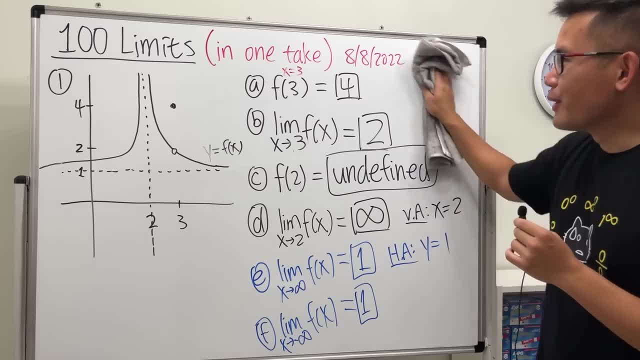 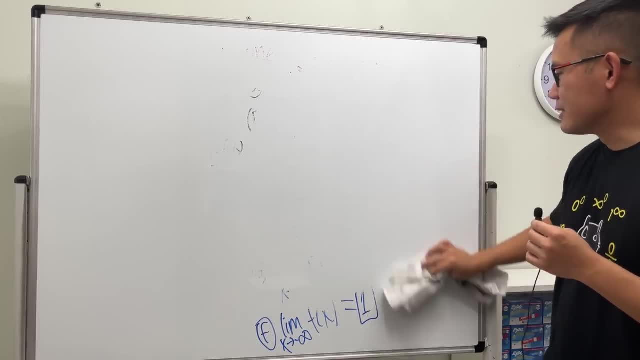 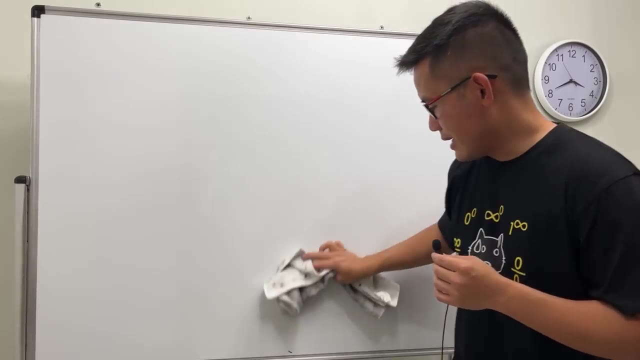 more to go and um, yeah, so let me just erase this. um, for the first couple questions, just maybe use the timestamp to navigate, especially, uh, because i will have to take some time to graph the function. so, yeah, i'll try to. i'll also try to give my best graph possible for you guys. 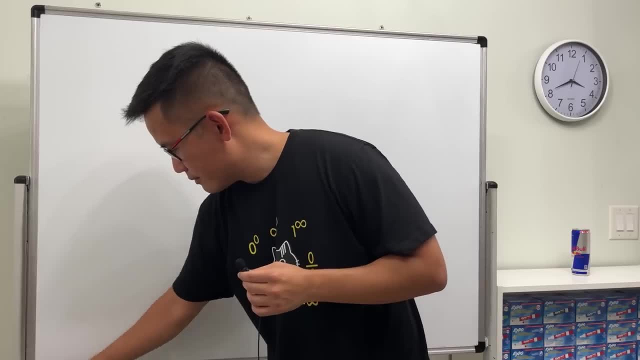 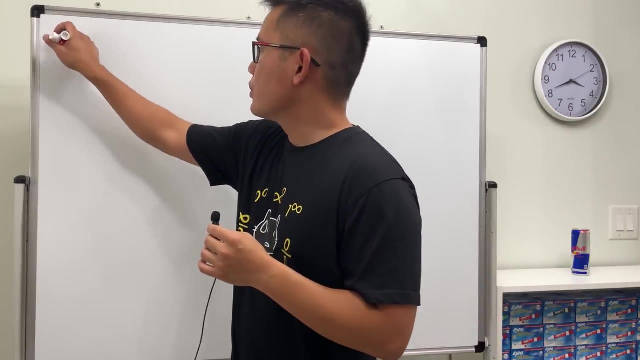 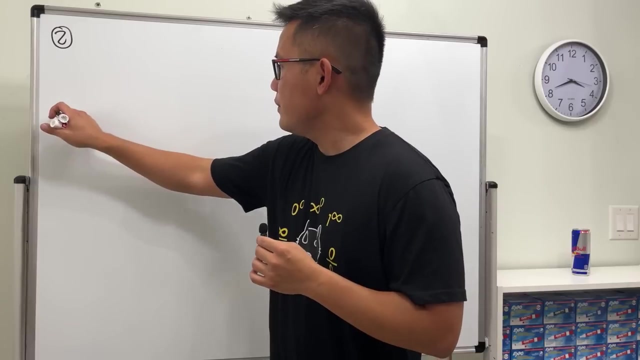 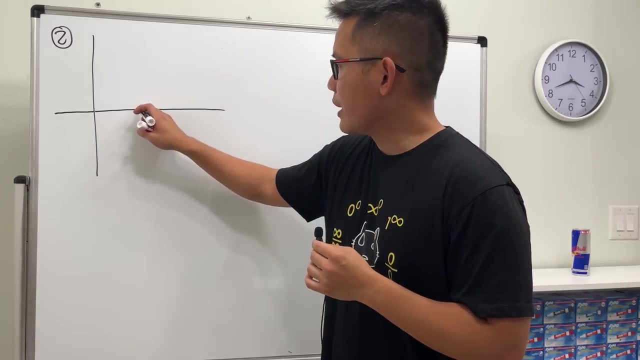 on the board. let me see if i can. there we go. okay, number two. all right, number two again. look at the file. my much better that way. anyway, i'm just gonna give you guys the important values. so here we have a two right here. of course that will be important and you'll see that. 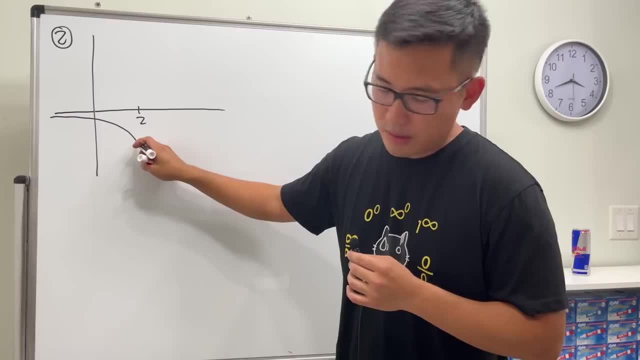 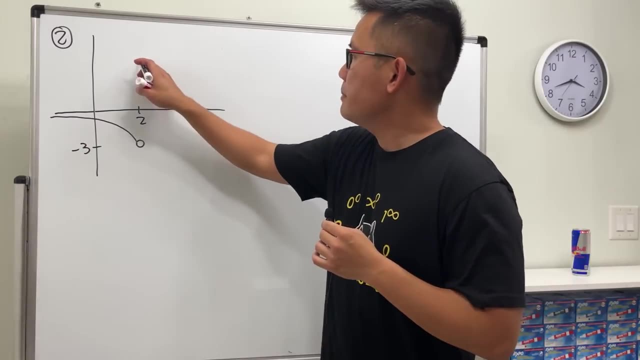 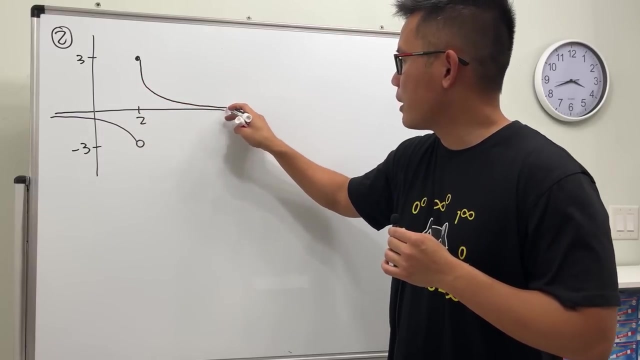 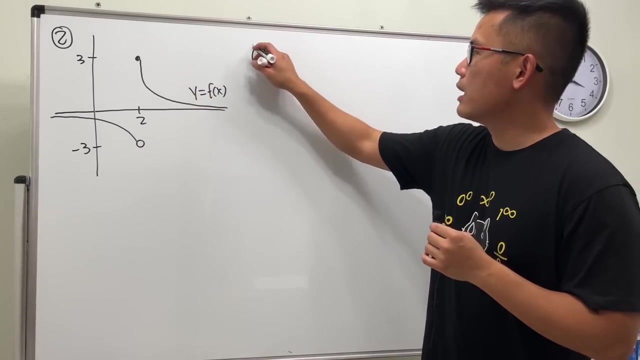 the curve looks like this, and then we have an open circle here and this is at negative three, and then, when we have, the other piece is up here, and then we have a closed circle and then we have this part, and of course this is our function. um couple parts first, part f of two. let's do this. 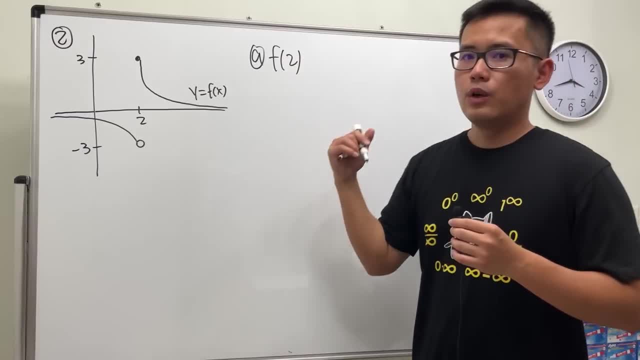 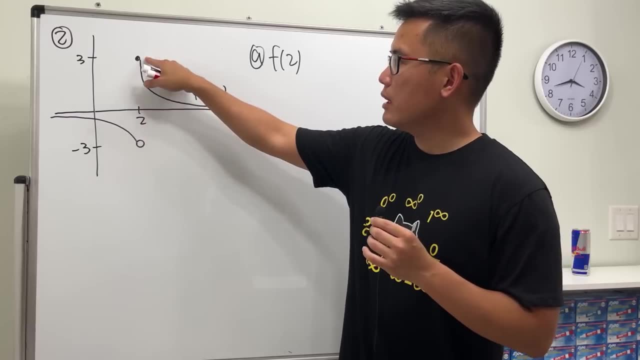 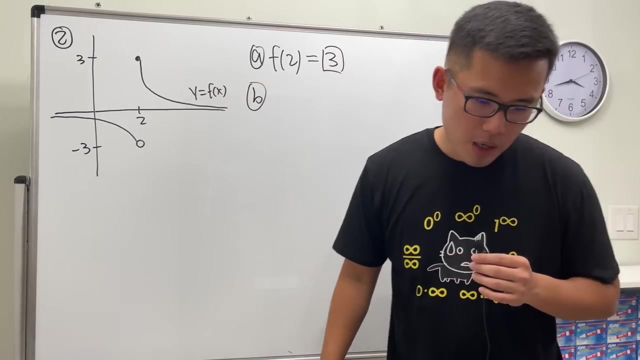 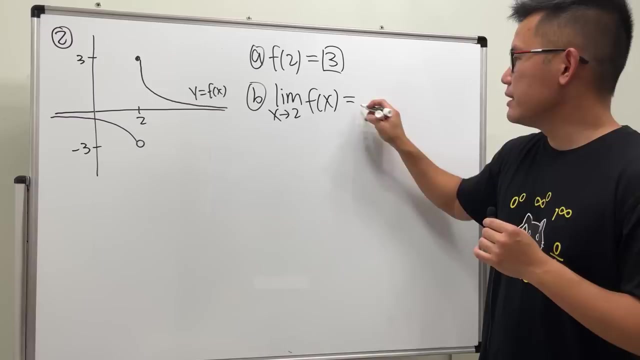 first. so this means when x is exactly equal to two, go here and look at the closed circle. so up here and look at the y value. three done f of two equals three, and you guessed it. part b: we will have the next one limit as x approaching two. this right here is going to be slightly different than the ones that 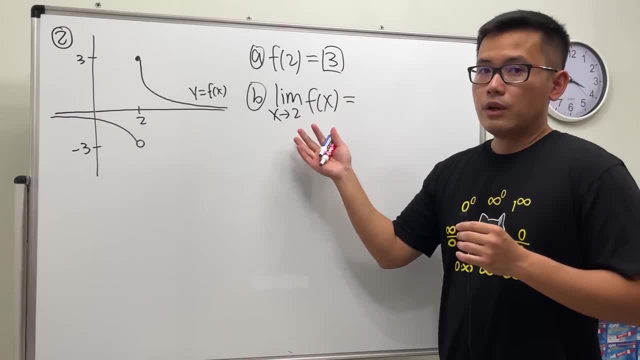 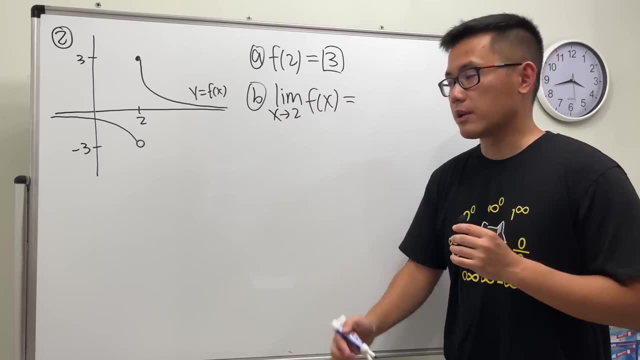 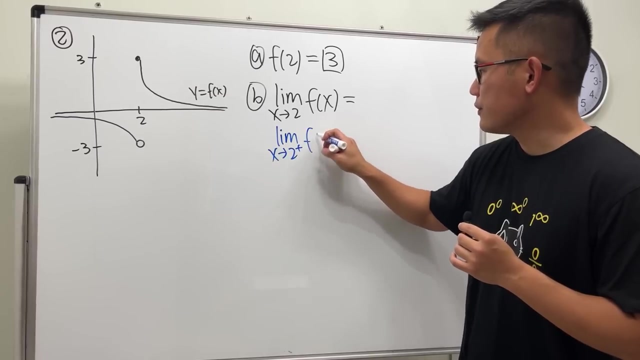 we did from the first question. firstly, we will have to again do the plus or minus on the side, because you didn't have that, so you really have to check both. so before we answer this question, let me just do this in blue: what's the limit as x approaching two? let's do the positive version first. 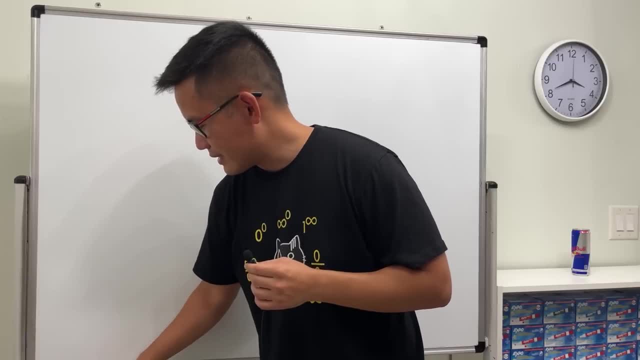 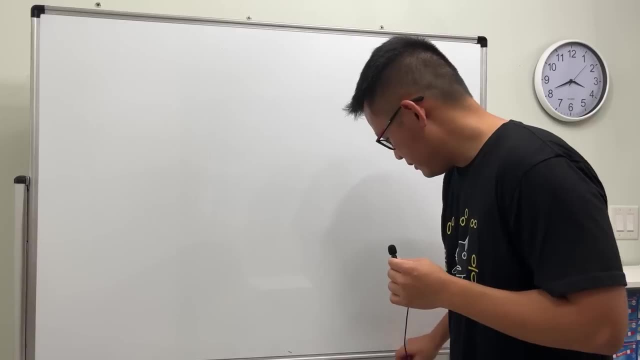 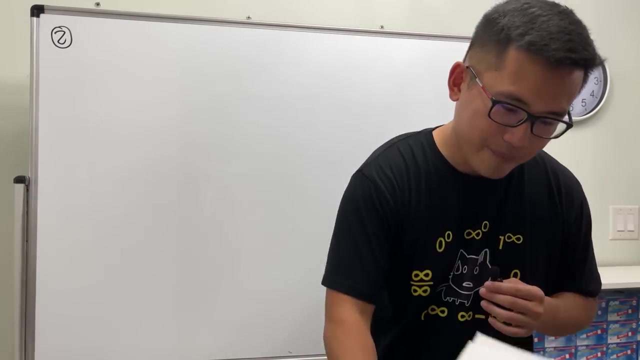 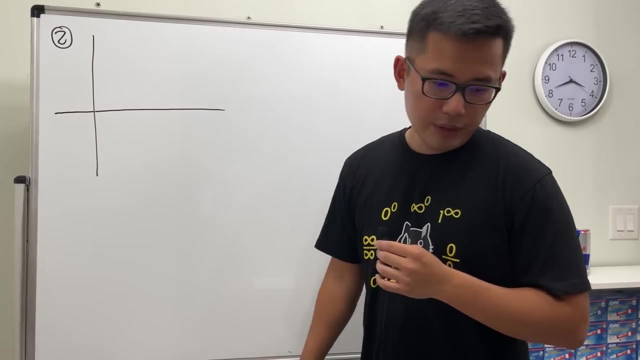 try to give my best graph possible for you guys on the board. let me see if I can. okay, number two. all right, number two. two again. look at the fire. much better that way. anyway, I'm just gonna give you guys the important values. so here we have a two, right here, of course that. 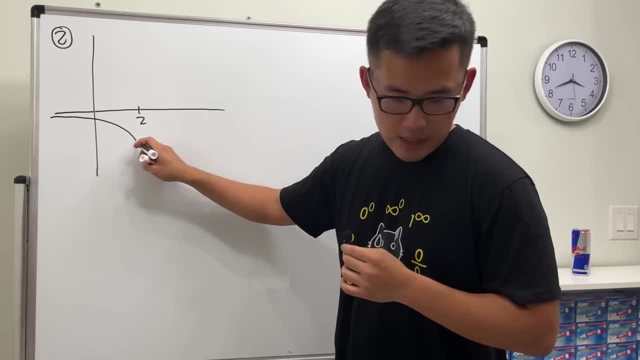 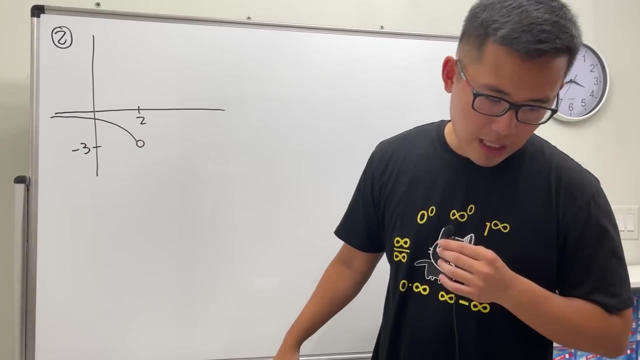 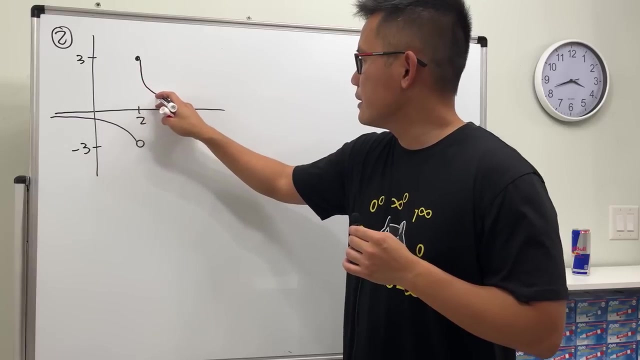 will be important and you'll see that the curve looks like this, and then we have an open circle here and this is at negative three, and then, when we have, the other piece is up here, and then we have a closed circle and then we have a COMPOSITE. 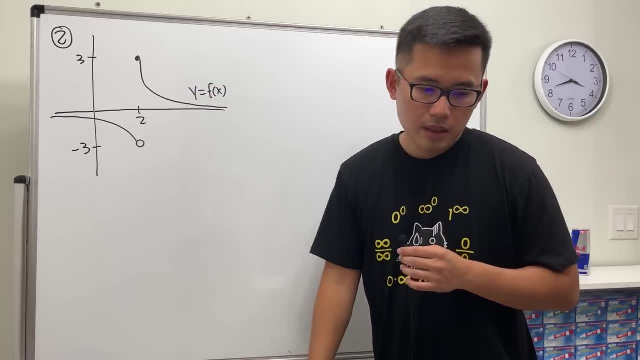 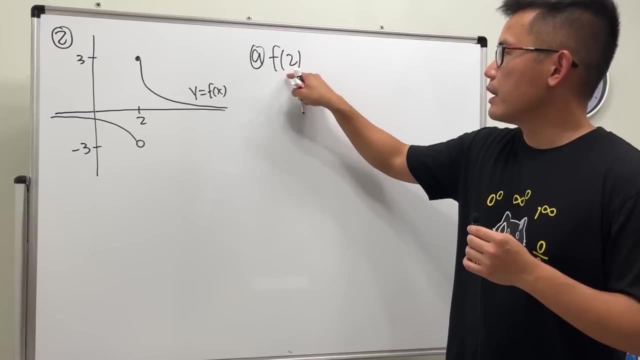 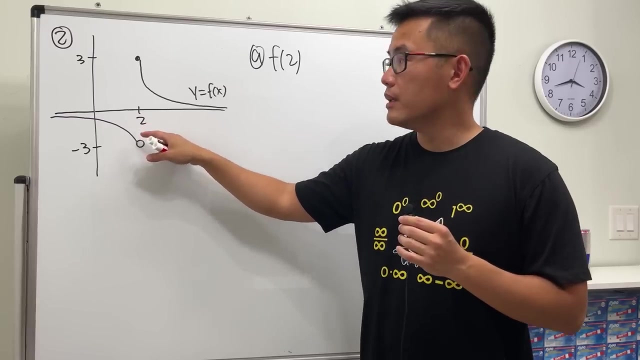 so let's do this again. so it's going to be initial function, so this is the thing that's important. so I want to make sure that I'm not forgetting about where I put thisرthis part, and of course, this is our function. erm couple parts. first part of two. let's do this first. so this means when X is exactly equal to 1end, T1t. 2 to 2nd. so this means when X is exactly equal 2nd. go here and look at the and look at the. go here and look at the Closed Circles. so up here and look, avoid all U. 3 done a fo 2 equals 3 and you guess if part B we will. 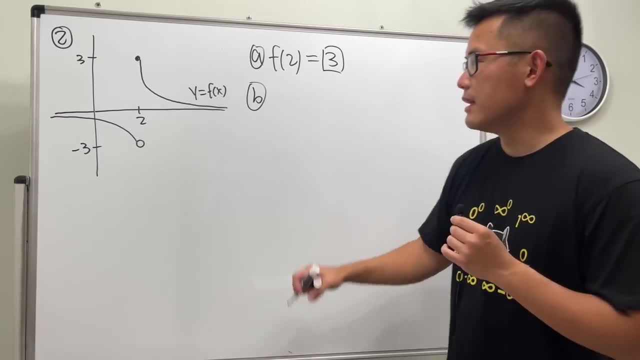 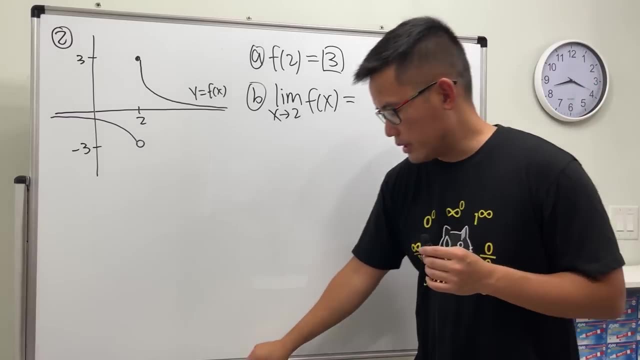 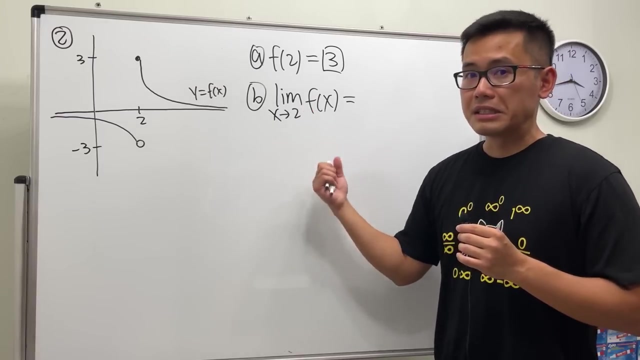 of 2 equals 3, and you just did Part B. we will have the limit as x approaching 2. this right here is going to be slightly different than the ones that we did from the first question. firstly, we will have to again do the plus or minus on the 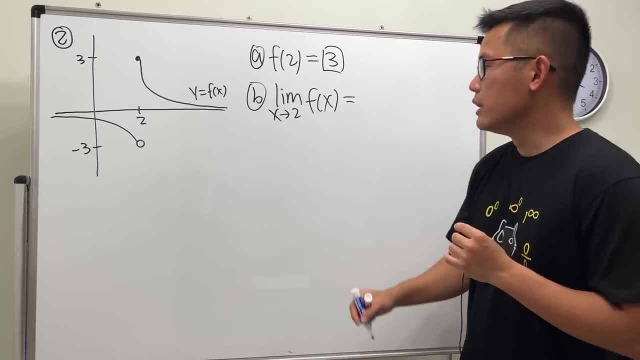 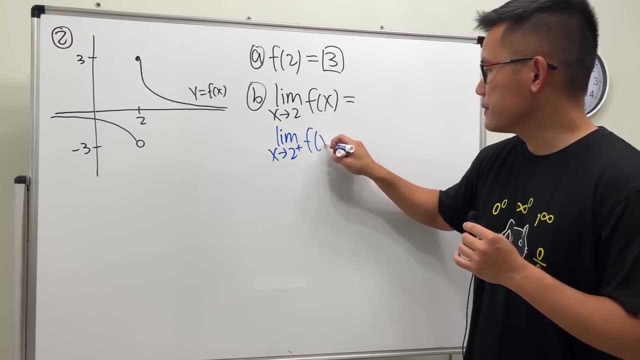 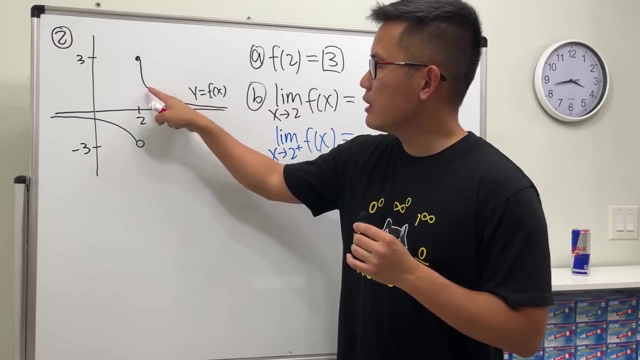 side, because it didn't have that. so you really have to check both. so before we answer this question, let me just do this in blue: what's the limit as x approaching 2? let's do the positive version first. so in this case we are approaching 2 from the right. so we see: okay, the y-file is. 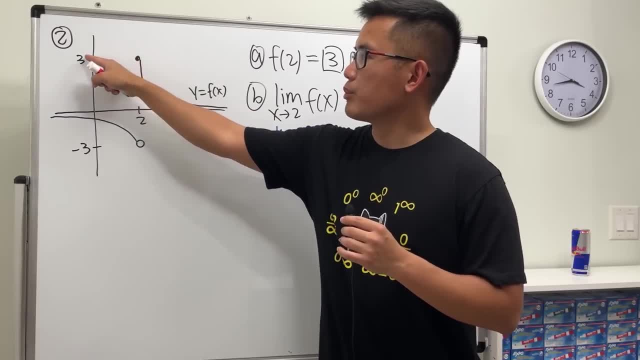 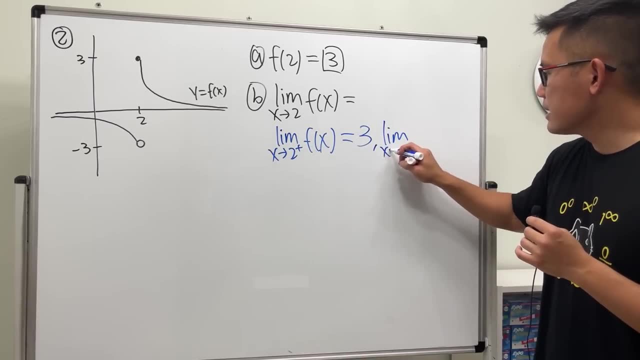 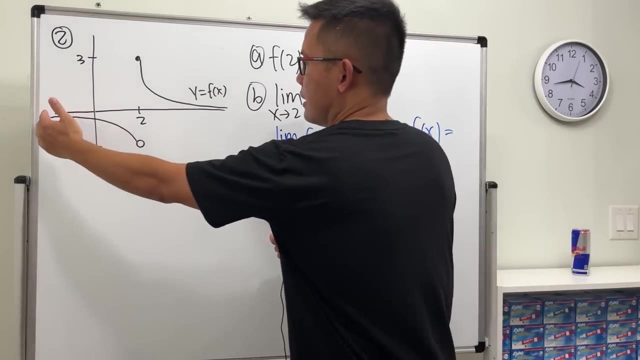 approaching 3, right, so just kind of look at this. and then approaching 3, so this is 3. however, if you look at the limit as x, approaching 2 minus, meaning from the left hand side, just left hand, right, starting from here, and then just kind of go to 2, but you see the. 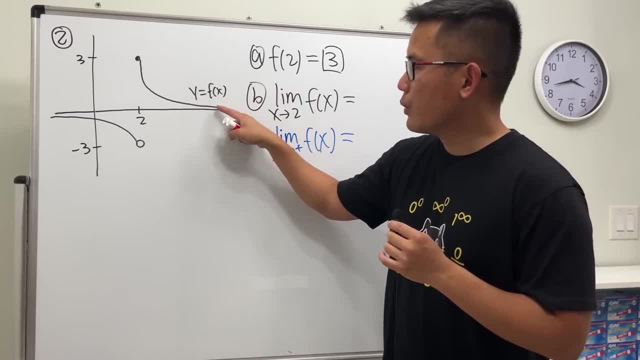 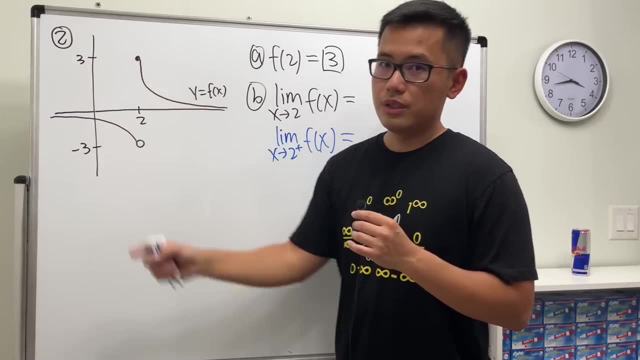 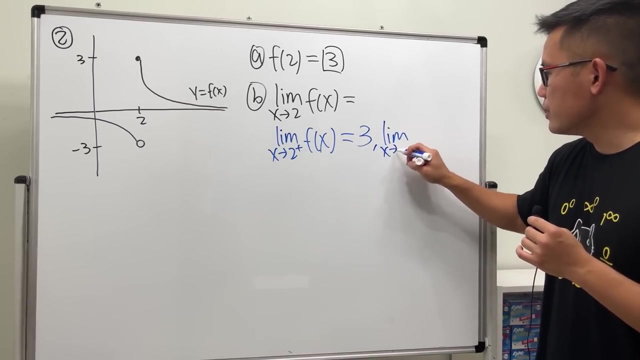 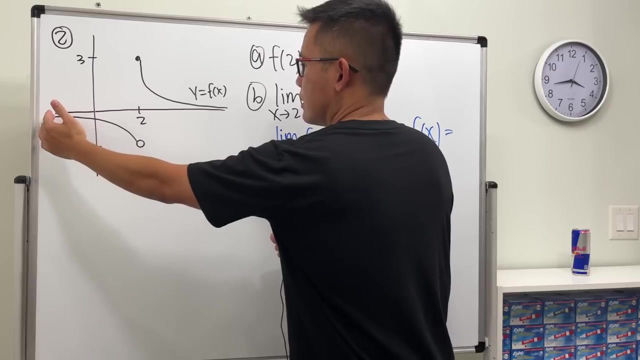 so in this case we are approaching two from the right. so, if you see, okay, the y-file is approaching three, right, so just kind of look at this and then approaching three, so this is three. however, if you look at the limit as x, approaching two, minus, meaning from the left hand side, just left hand, all right, starting from here, and then just kind of go. 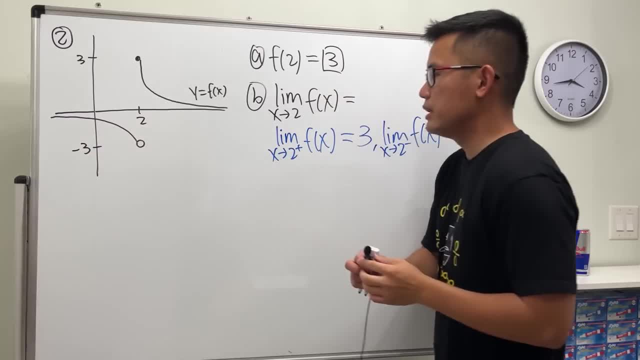 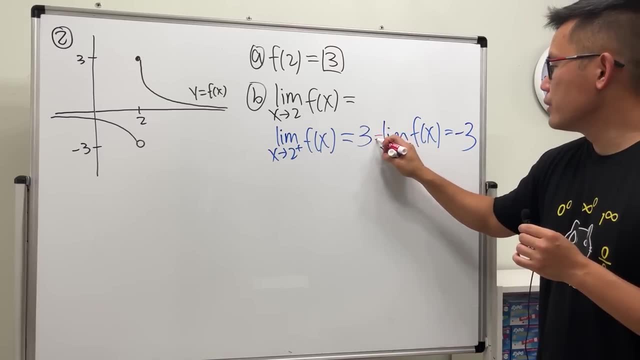 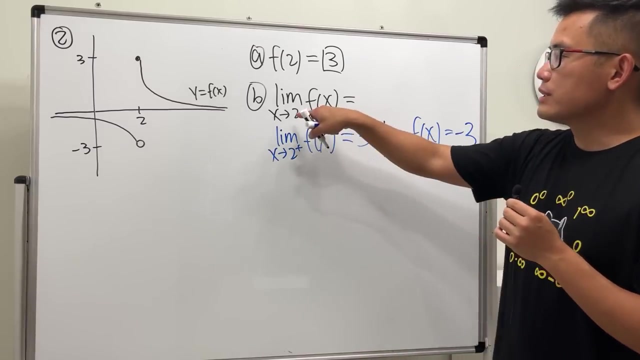 to two, but you see the y-file is approaching negative three, so this right here will give us negative three. that three is not equal to negative three. therefore, the answer for this: we do not have the answer and again, just like what i said earlier, when we are talking about limits, the way that 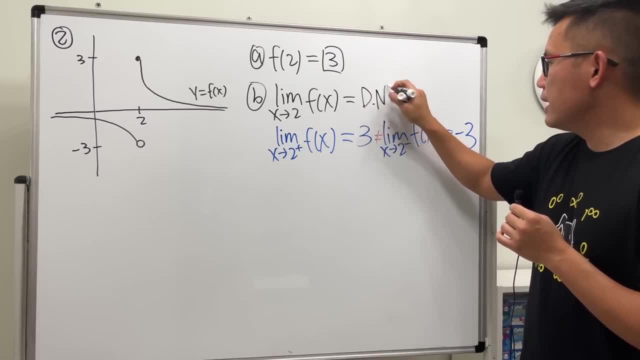 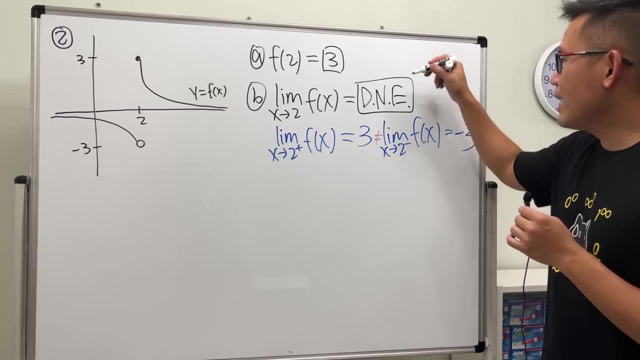 we answer is: does not exist. so i'll just put on d and e. i really don't know why i like to put on dots, but anyway i'll spell this out at least one time. this abbreviates does not exist, and the reason that we really say it does not exist is because when we ask the limit we like to ask. 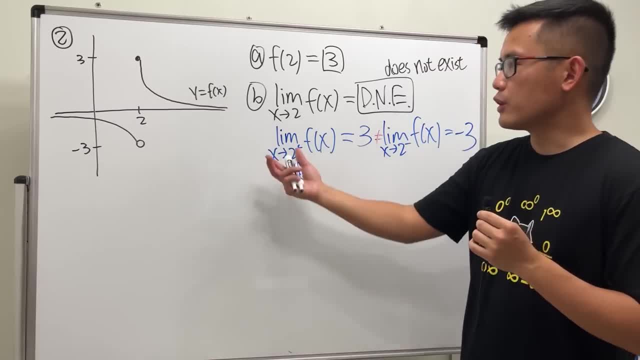 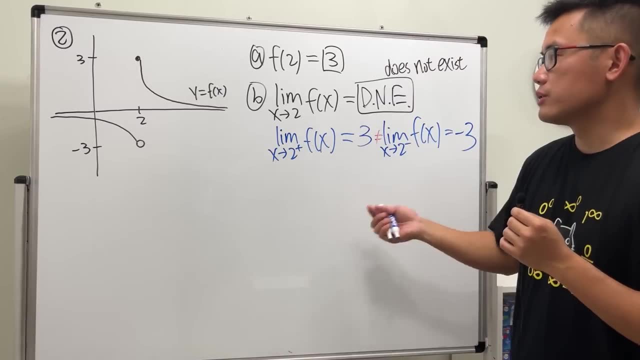 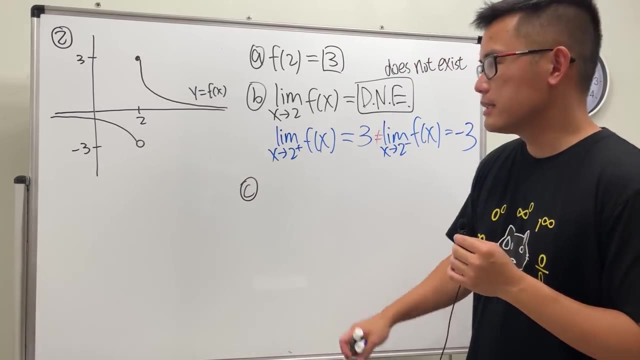 is there a number or does there exist a number that the function is approaching when x is approaching a certain number? if it's a no, then you answer: it does not exist. there is no such a number. so i think that's the reason why c limit as x approaching infinity. 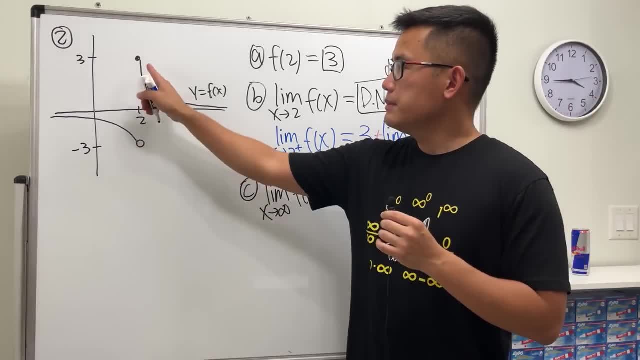 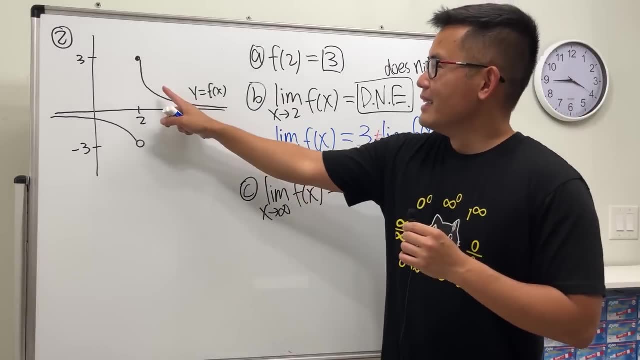 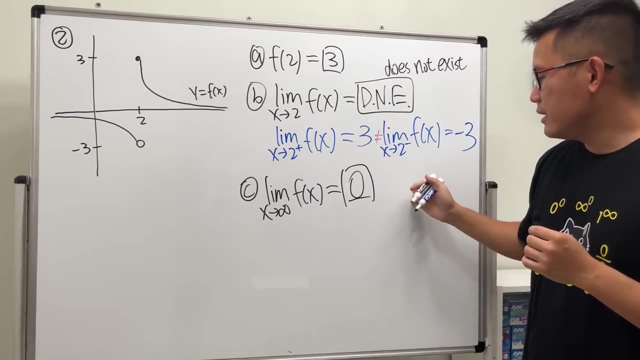 of the function. well, this means x is all the way to the right. and again, don't worry about this being like no, no, when the curve is like this, you see that the y bar is approaching zero. so, yeah, this is zero. and then, if the question also asks you for like, okay, what's the horizontal arsenal? 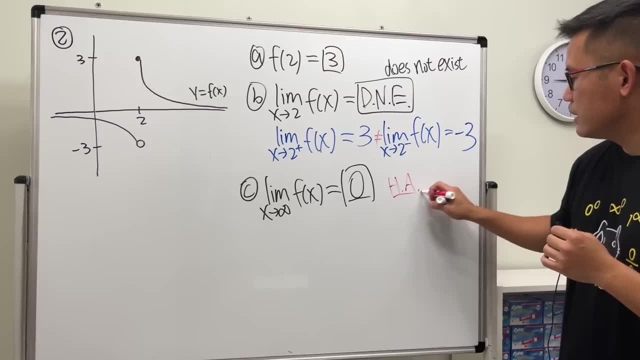 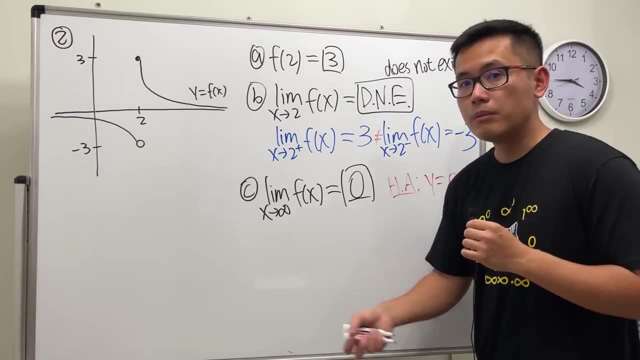 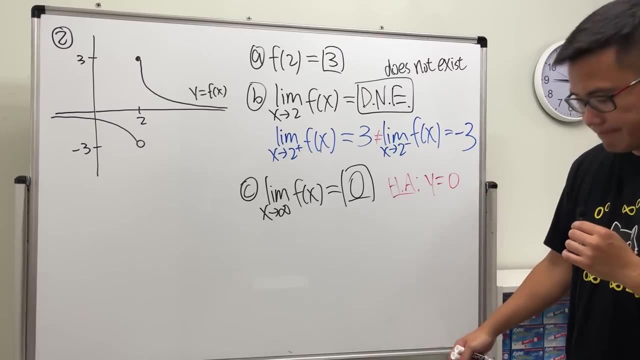 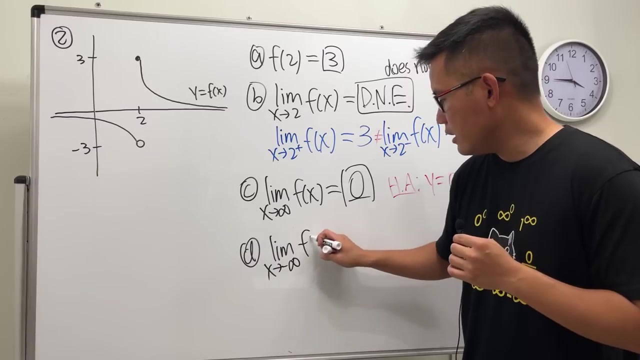 from here can say: the horizontal arsenal is y equals zero, right. so if the question is asking us for limit, we get zero. or if the question is asking us find the horizontal arsenal, we do that, and then we say y is equal to zero, all right. the limit x, approaching negative infinity of the function. 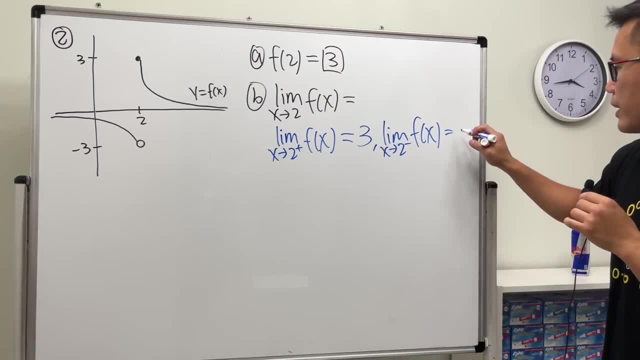 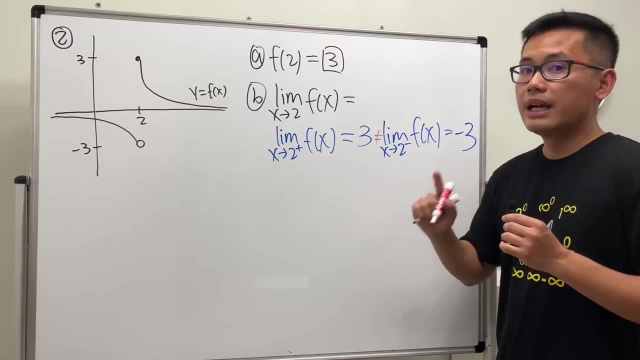 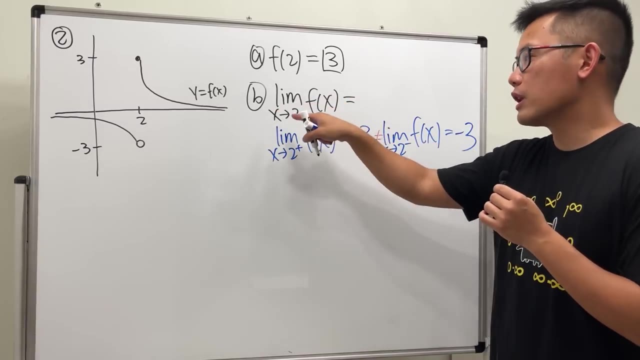 y-file is approaching negative 3, so this right here will give us negative 3 and notice that 3 is not equal to negative 3. therefore, the answer for this: we do not have the answer and again, just like what i said earlier, when we are talking about limits, the way that we answer, 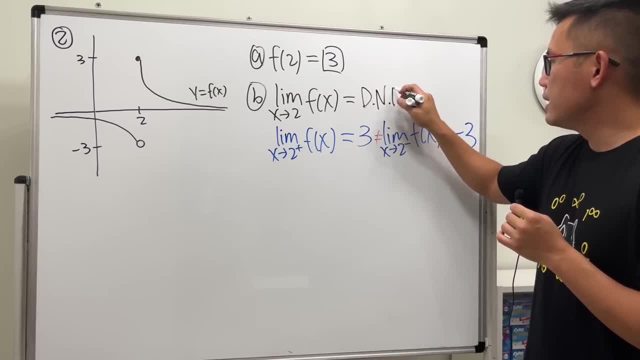 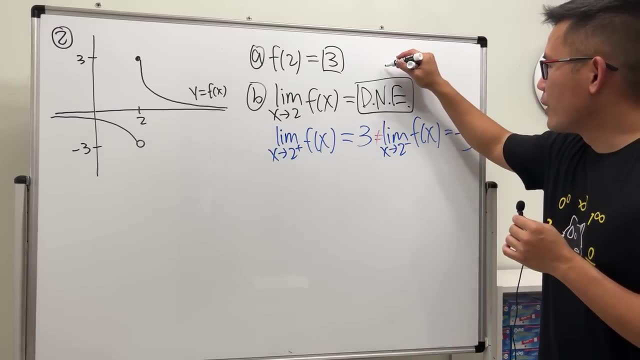 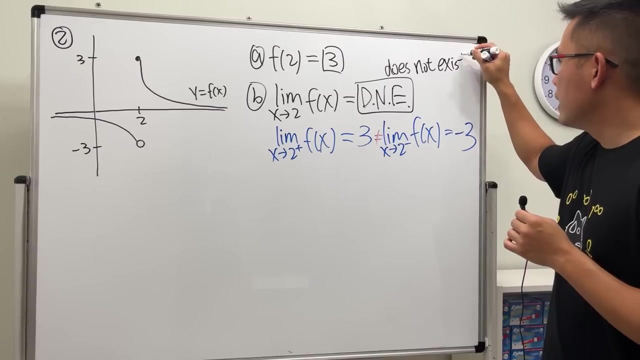 is does not exist, so i'll just put on d and e. i really don't know why i like to put on dots, but anyway i'll spell this out at least one time. this abbreviates does not exist and the reason that we really say it does. 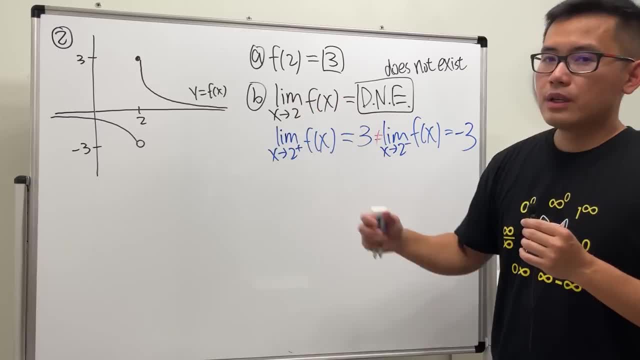 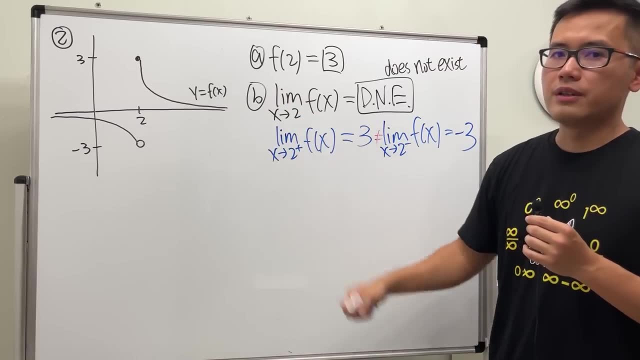 not exist is because when we ask the limit, we like to ask: is there a number or does there exist a number that the function is approaching? when x is approaching a certain number, if it's a no, then you answer: it does not exist. there is no such a number. so i think that's. 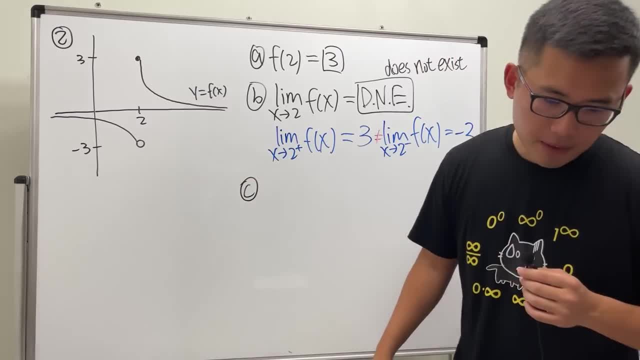 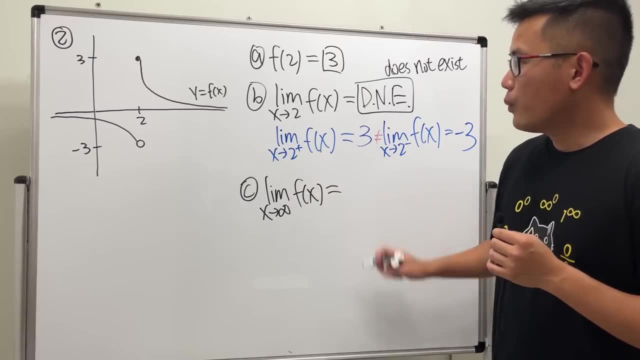 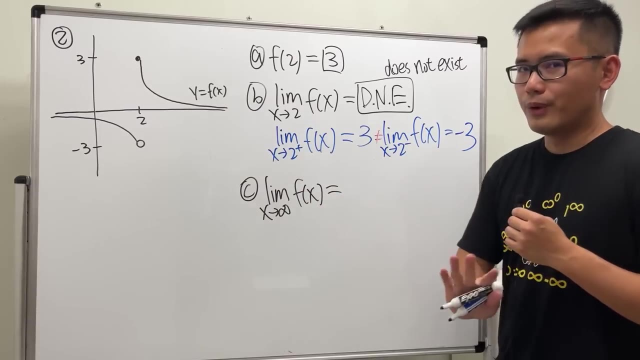 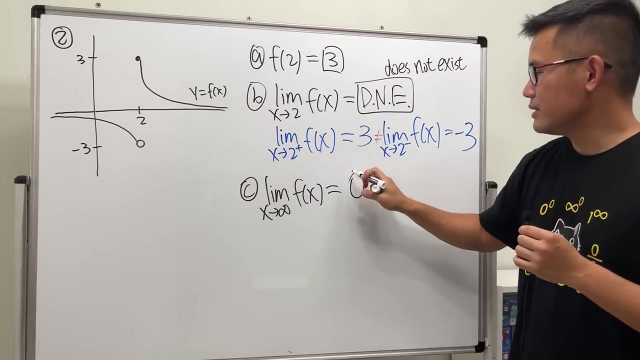 the reason why c limit as x approaching infinity of the function. well, this means x is all the way to the right and again, don't worry about this being like. when the curve is like this, you see that the y-file is approaching zero. so, yeah, this is zero. and then, if the question 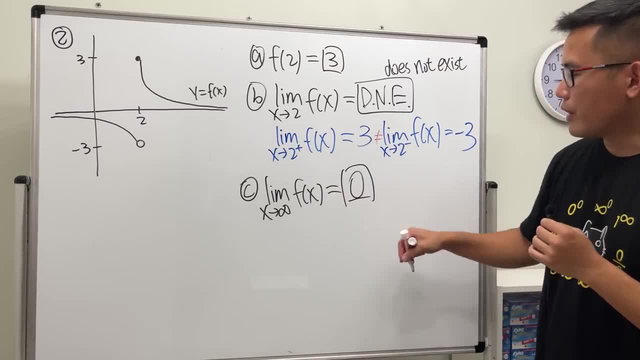 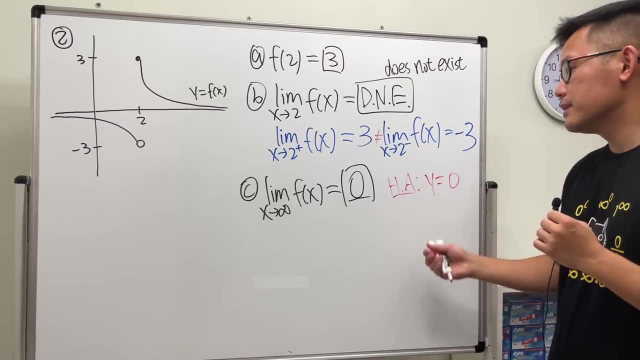 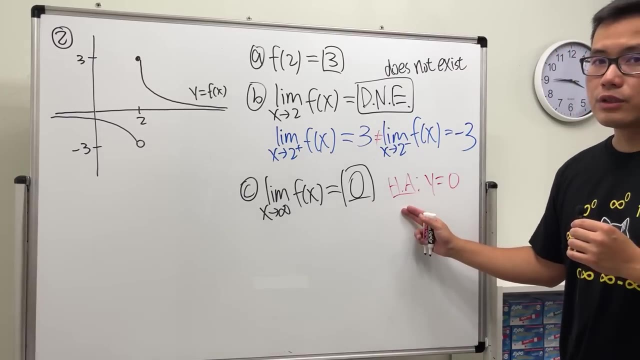 also asks you for: like: okay, what's the horizontal acetal? from here we can say: the horizontal acetal is y equals zero, right? so if the question is asking us for limit, we get zero. or if the question is asking us find the horizontal acetal, we do that and then we say y is equal. 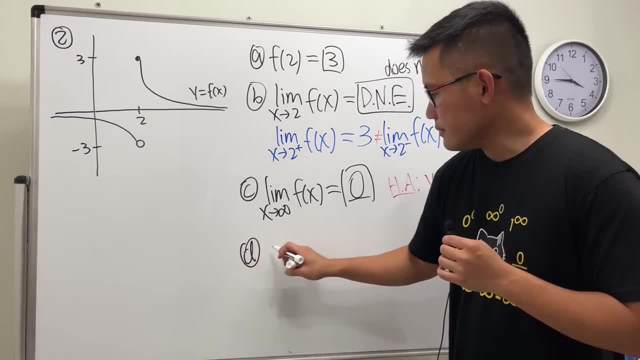 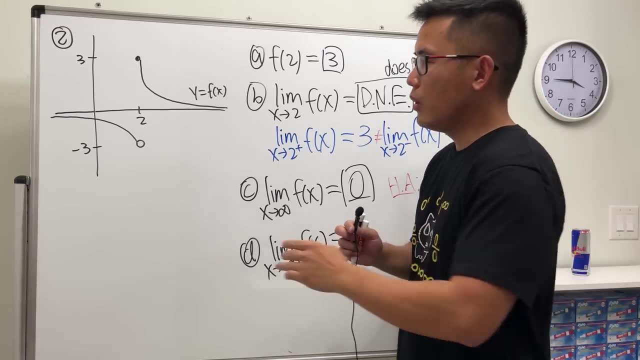 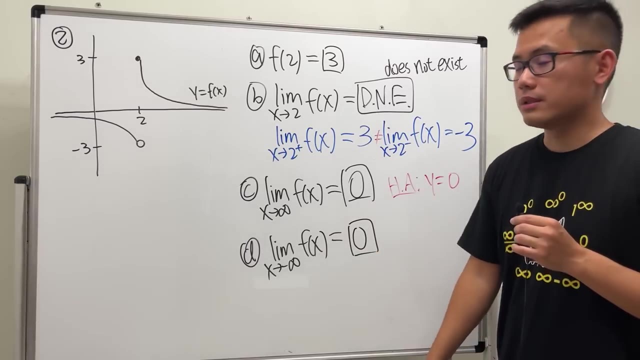 to zero, all right. the limit x approaching negative, infinity of the function. this means we go all the way to the left and the y value is approaching zero, and you do not have to write the horizontal acetal twice because they are the same right? so, yep, that is number two, and then again, we just 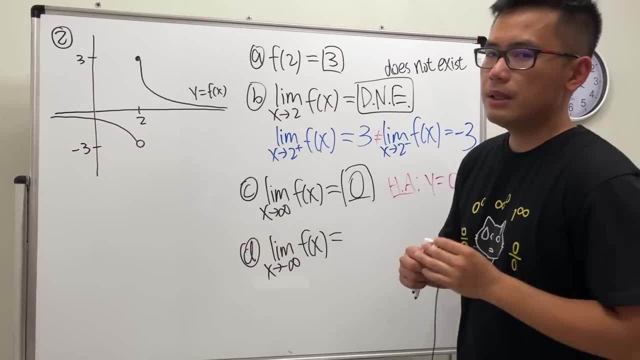 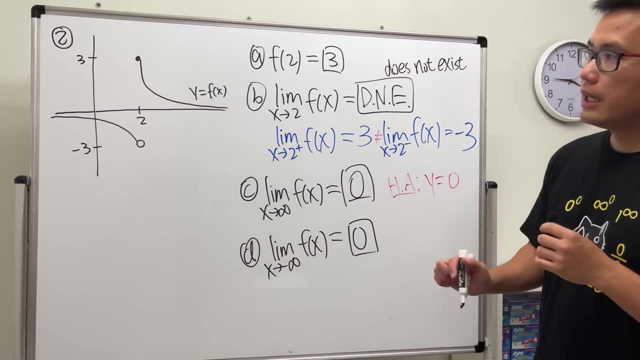 this means we go all the way to the left and the y value is approaching zero, and you do not have to write the horizontal twice, because they are the same right. so yep, that is number two, and then again, we just have a couple more to go. 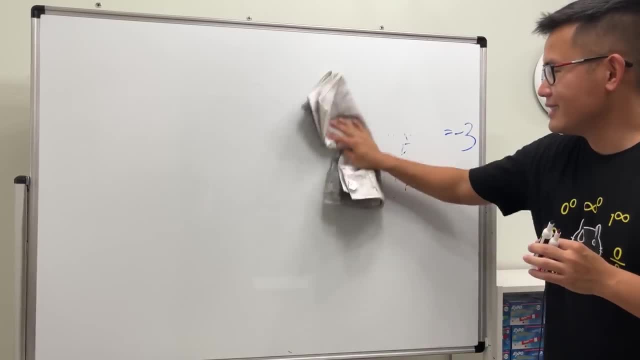 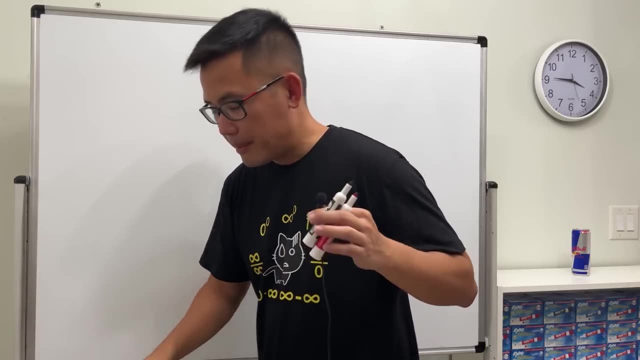 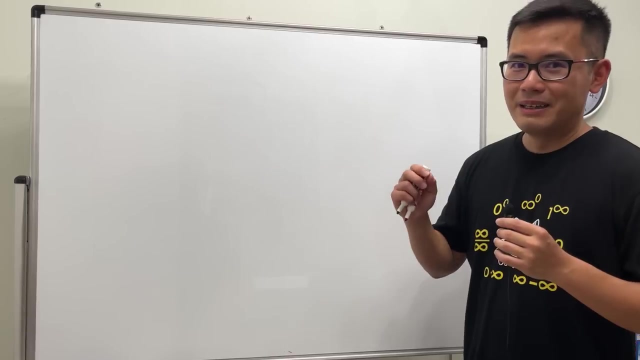 how are you guys doing? are you guys taking your calc one or call two classes? let me know. and, uh, i'm going to check, yeah, periodically, because i'm using my phone. i want to check. what does that mean? i need to check, want to make sure that, uh, my phone is recording and uh, i'm also charging it. hopefully nothing goes. 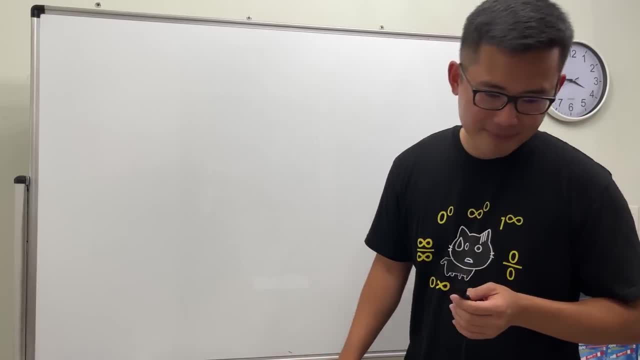 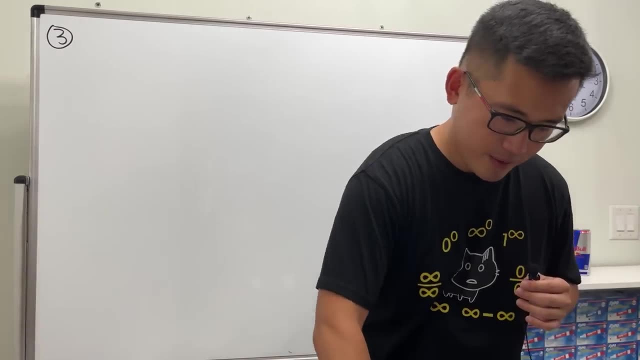 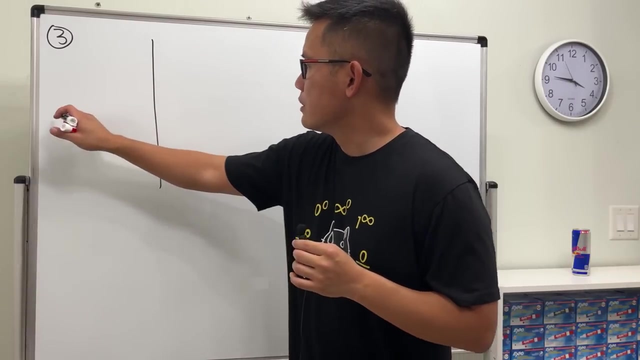 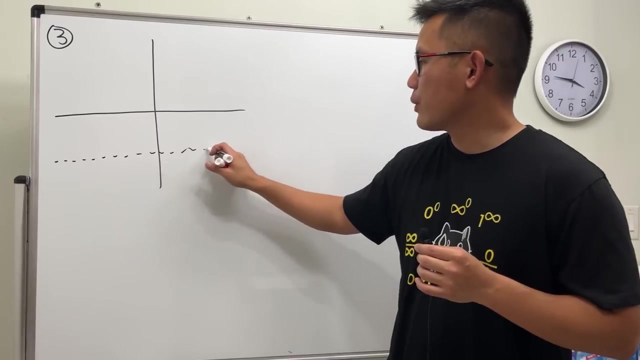 wrong. yeah, anyway, though, number three, this right here looks slightly weirder or more weird, anyway, okay. so here is the picture. firstly, i will give you guys the horizontal as the hopes. inside we have a horizontal dash line here, and then likewise here- this is going to help me to draw the pictures- and then we have a 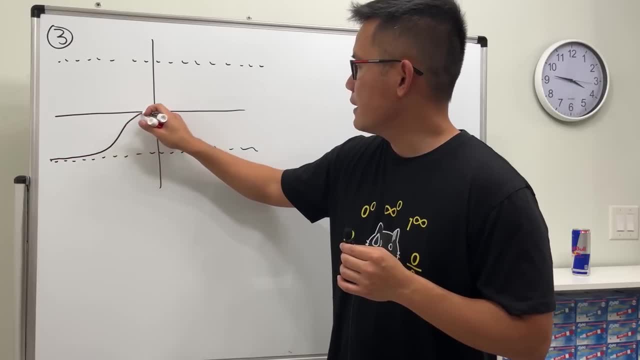 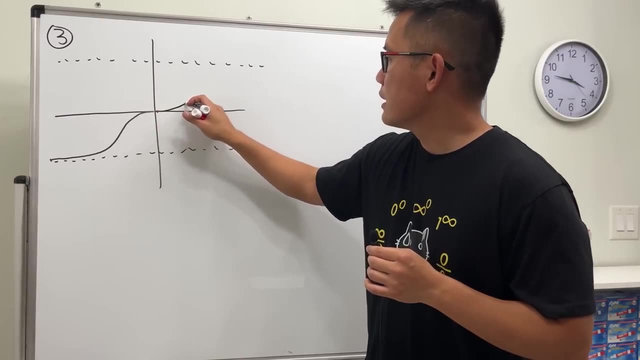 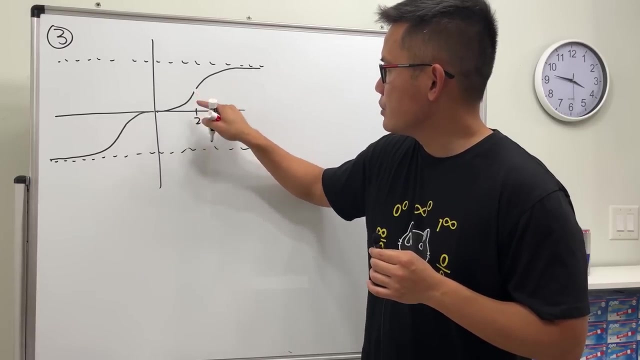 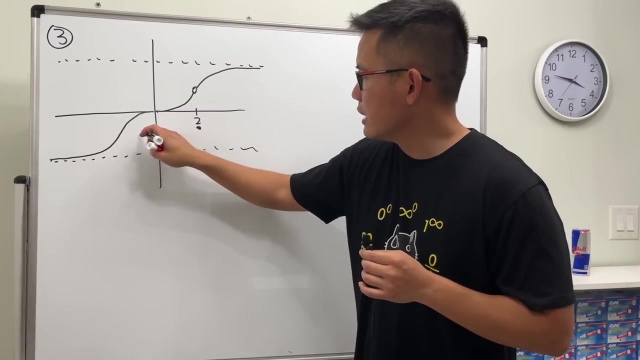 curve goes like this and up and then flex, and then okay, and then flag, and then like this and then like so, and when let's say here is two, and then let me just get rid of that, and then we have a closed circle here, and the void for the closed circle is: 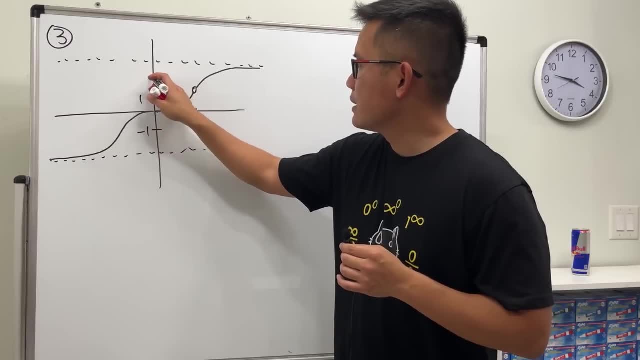 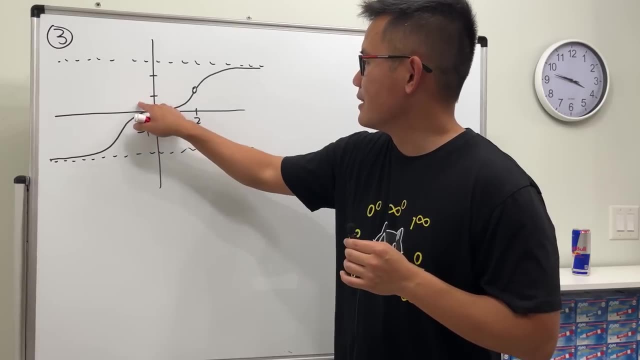 negative one, and then here is one, and then here is- actually, i will just tell you, because my picture is going to be really bad- so, yeah, this right here is meant to be 1.5 and this right here is meant to be: y is equal to 2. 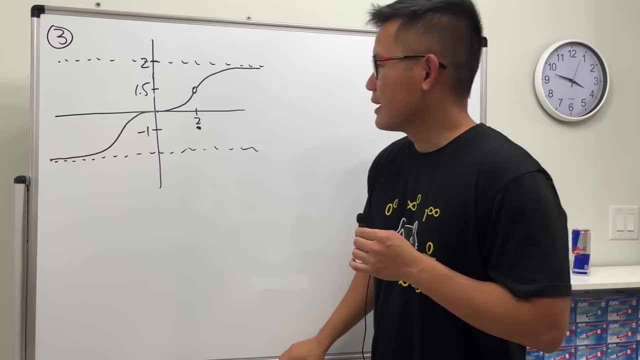 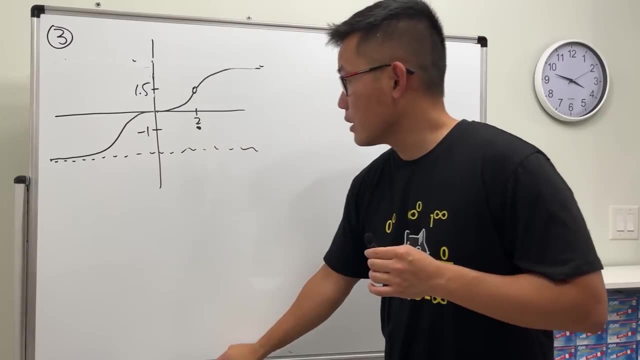 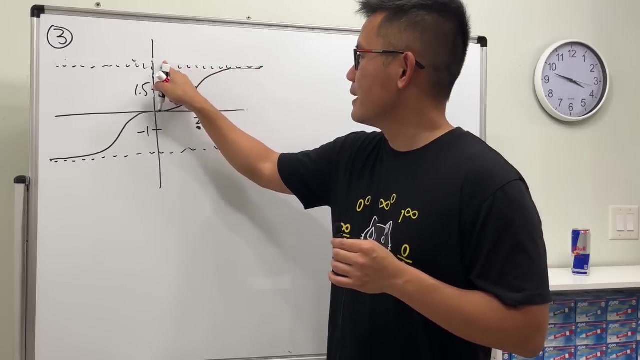 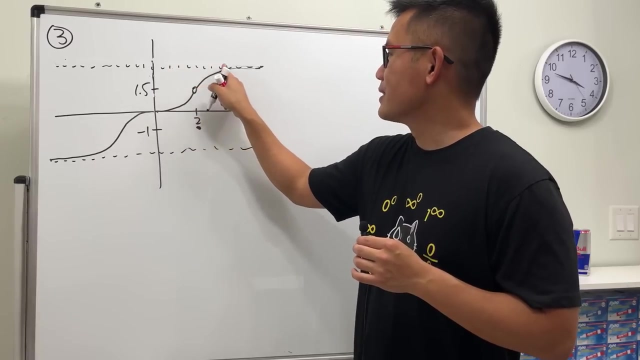 all right. so yeah, it's yeah. yeah, i'll try to fix it a little bit. okay, maybe slightly better, maybe worse. now this is worse. do you think i'm going to edit the video? no, i'm not, so just be patient and then use the timestamp to navigate, as i said, anyway, this right. here is two. right, this is horizontal. let's finish this. 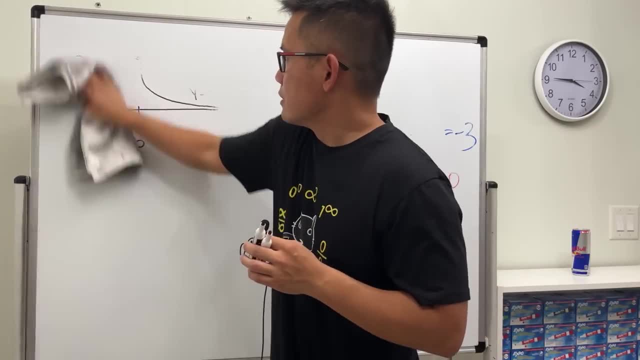 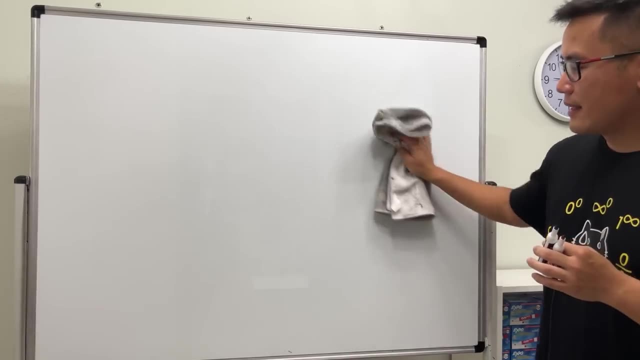 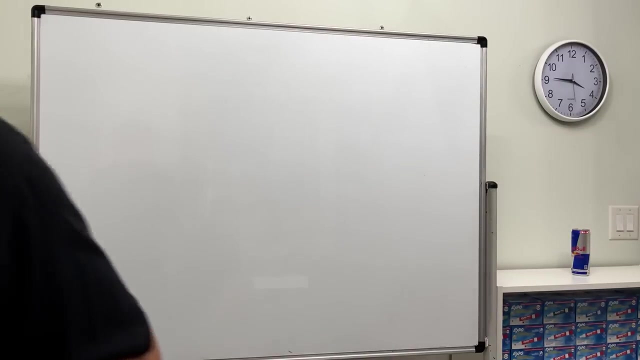 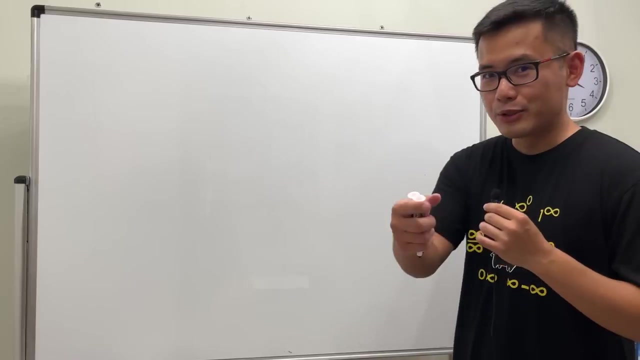 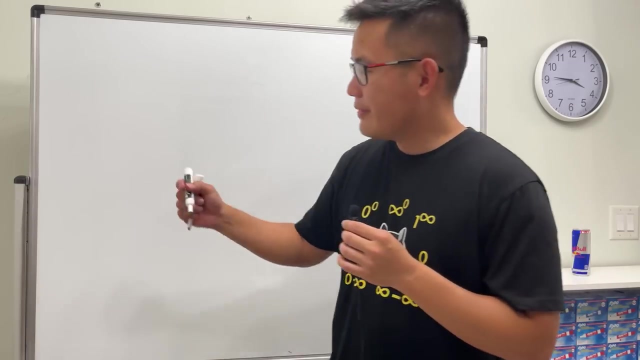 have a couple more to go. how are you guys doing? are you guys taking your calc one or calc two classes? let me know, and i'm going to check, yeah, periodically, because i'm using my phone. i want to make sure that, uh, my phone is recording and i'm also charging it. hopefully nothing goes wrong. yeah, anyway, though. number three: 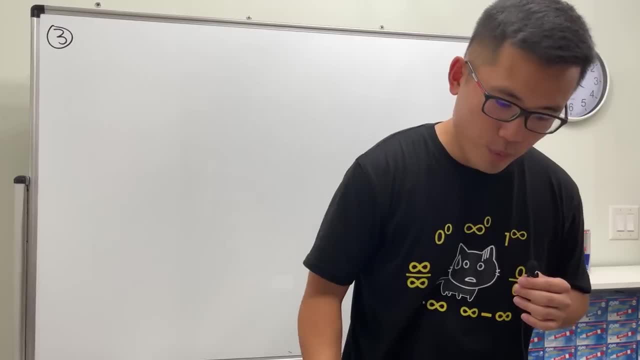 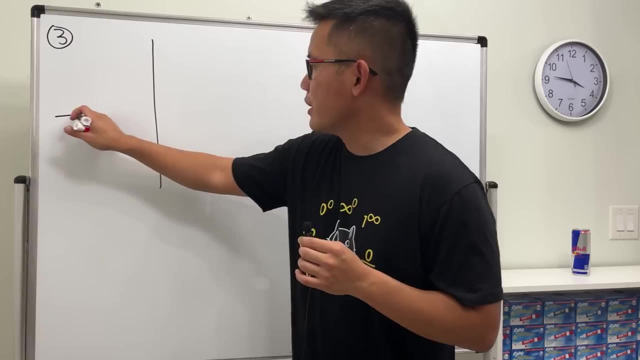 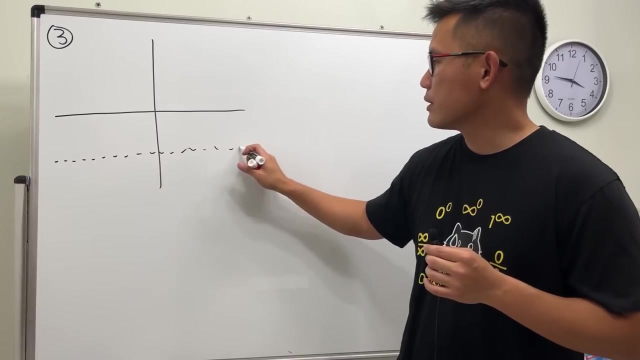 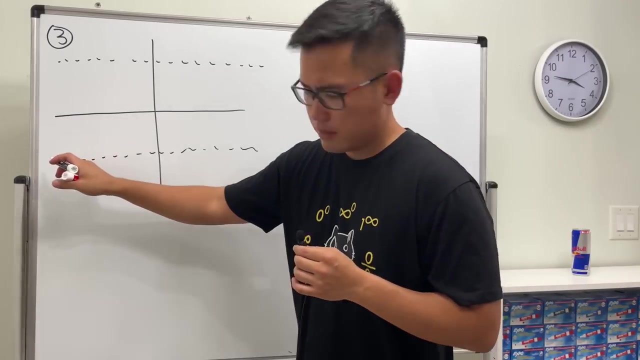 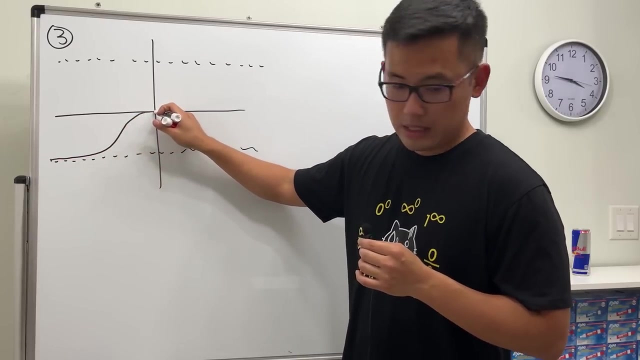 this right here looks slightly weirder or more weird, anyway. okay, so here is the picture. firstly, i will give you guys the horizontal as the hopes. inside. we have a horizontal dash line here and then likewise here- this is going to help me to draw the pictures- and then we have a curve goes like this and up, and then flex, and then. 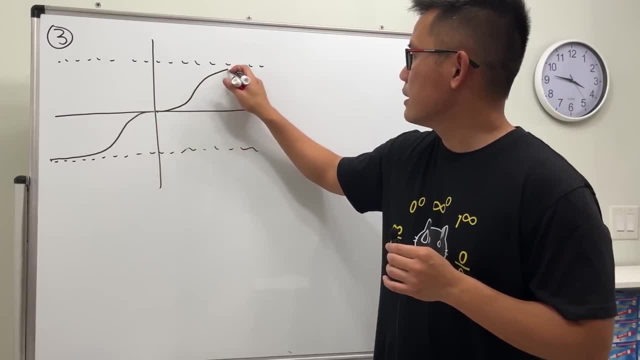 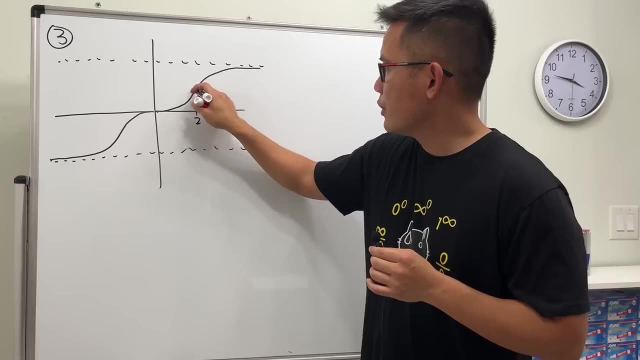 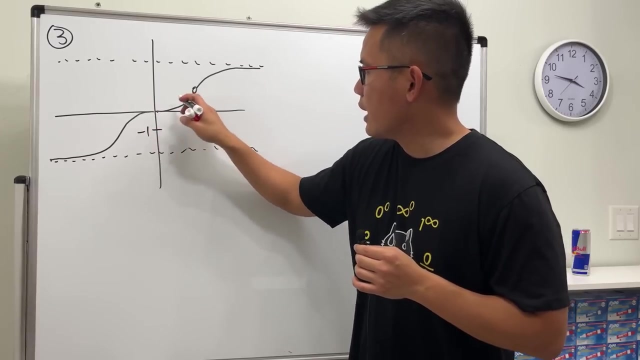 okay, and then flag, and then like this and then like so, and when let's say here is two, and then let me just get rid of that, and then we have a closed circle here and the void for the closed circle is negative one, and then here is one, and 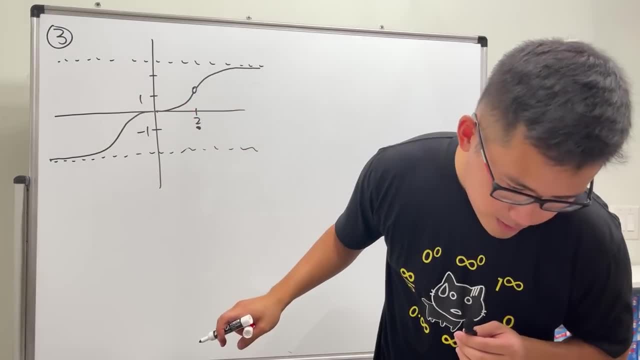 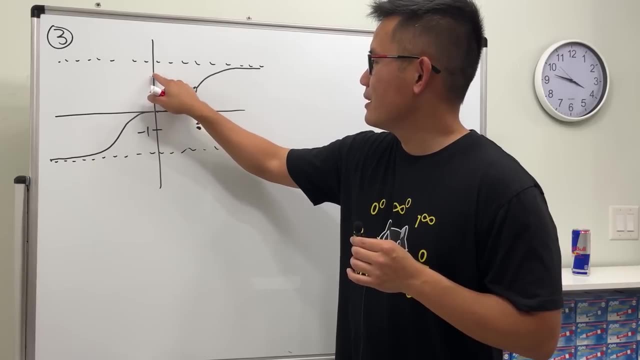 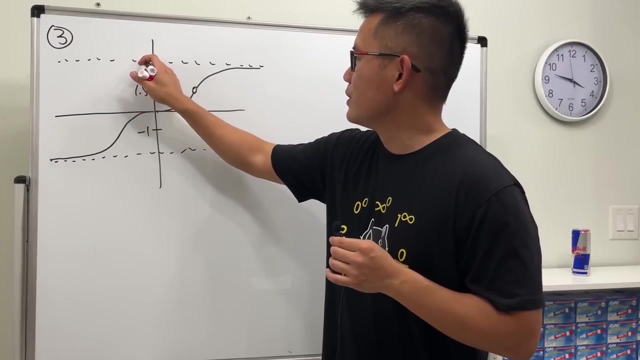 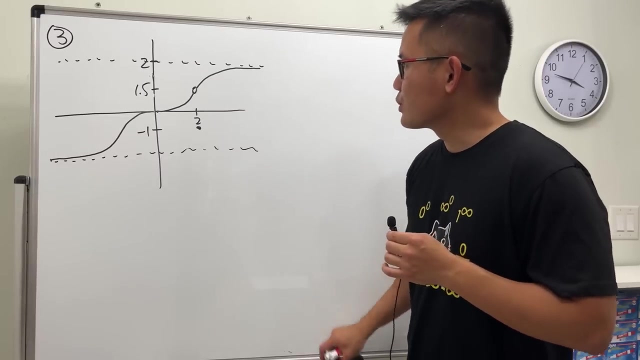 then here is actually i will just tell you, because my picture is going to be really bad. so yeah, this right here is meant to be 1.5 and this right here is meant to be y is equal to 2, all right, so yeah, i'll try to fix it a little bit. 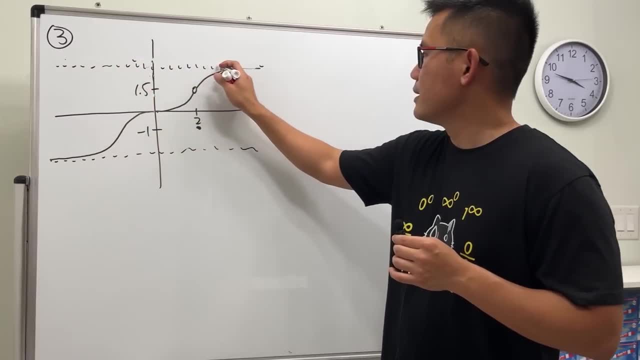 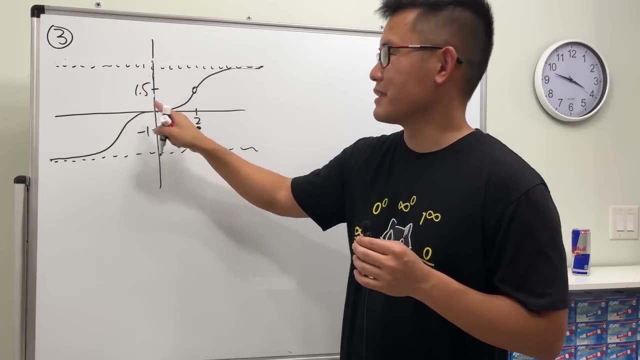 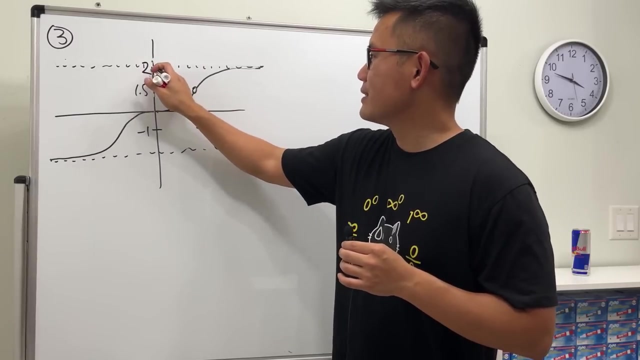 okay, maybe slightly better, maybe worse. this is worse. do you think i'm going to edit the video? no, i'm not, so just be patient and then use the timestamp to navigate. as i said. anyway, this right here is two. all right, this is horizontal. let's finish this creation as quickly possible, because the picture 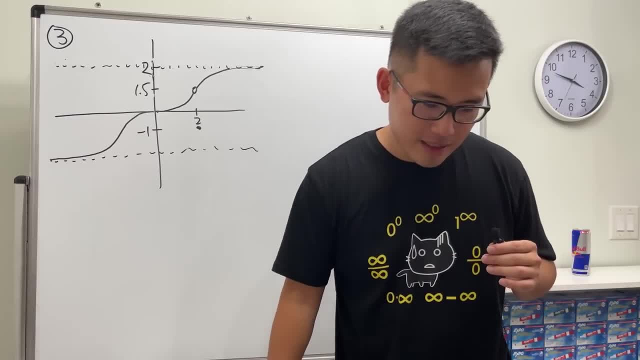 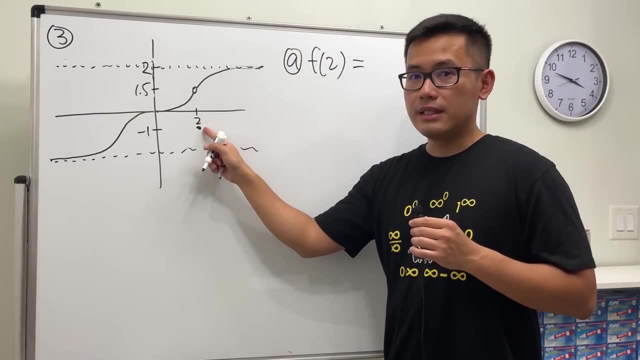 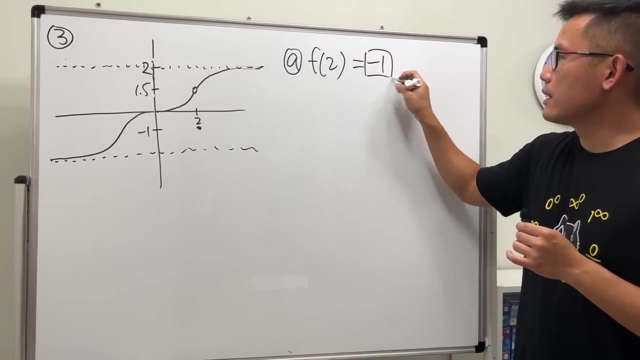 doesn't look nice. anyway, here is number three and um. first question, part a: what is the value for f of two? that means x is exactly two. you look at the y value, the dot right here, right, so it's negative one. so f of two is negative, one done b, you can guess it. what's the limit as x approaching two? 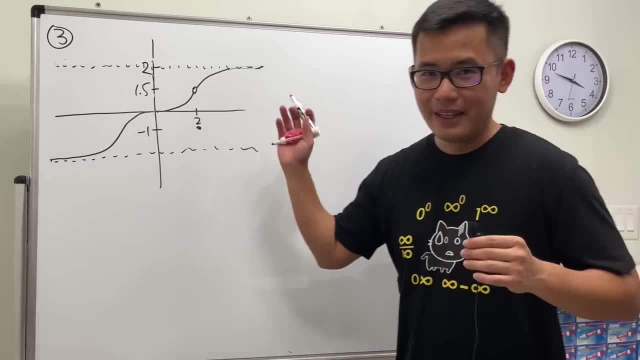 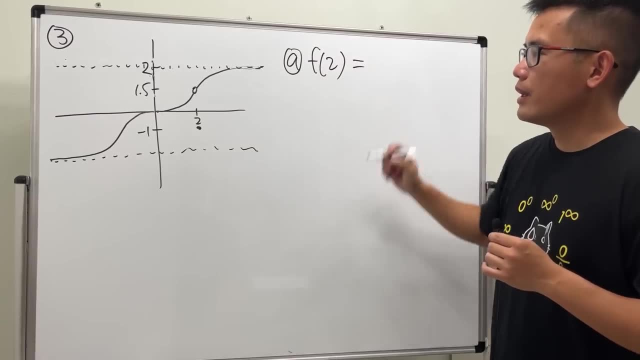 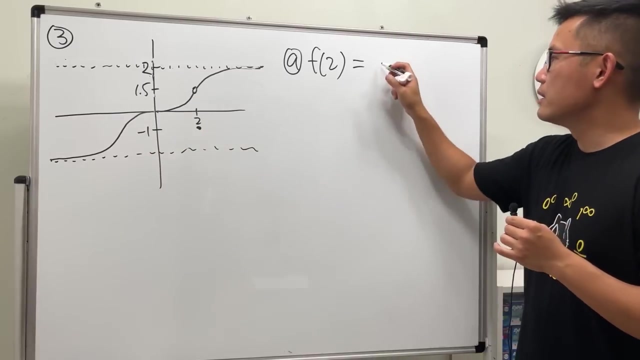 creation as quickly possible, because the picture doesn't look nice anyway. here is number three and the first question, part a: what is the value for f of two? that means x is exactly two. you look at the y value, the dot right here, right, so it's negative one. so f of two is negative one. done b, you can. 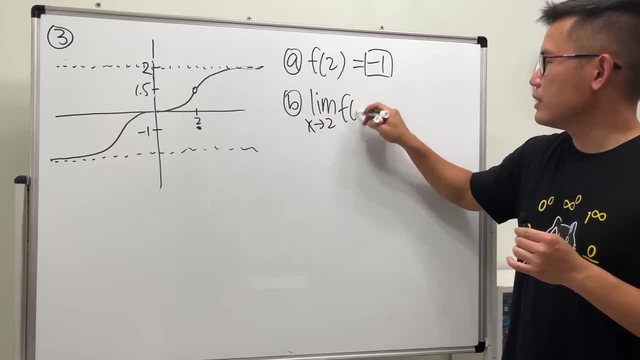 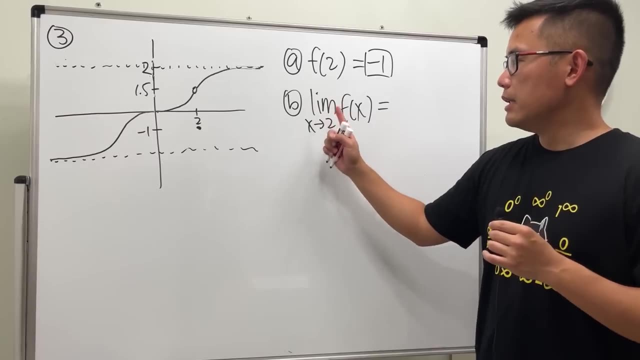 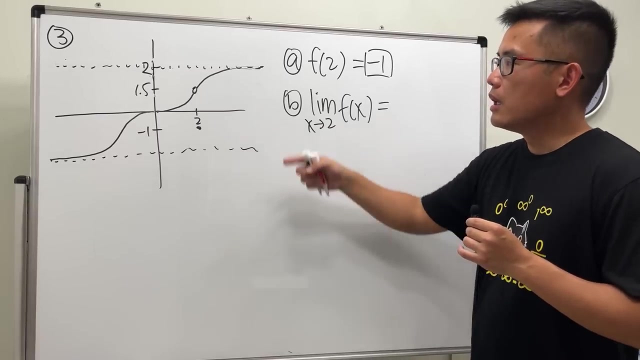 guess it, what's the limit as x approaching two of the function f of x? yeah, well, when we're talking about the limit as x approaching two, we do not care when x is exactly two, right? so the answer is actually not negative one, but rather you see how the curve is approaching what the wifi is. 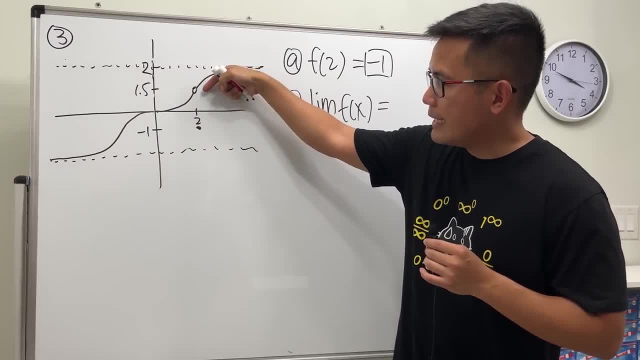 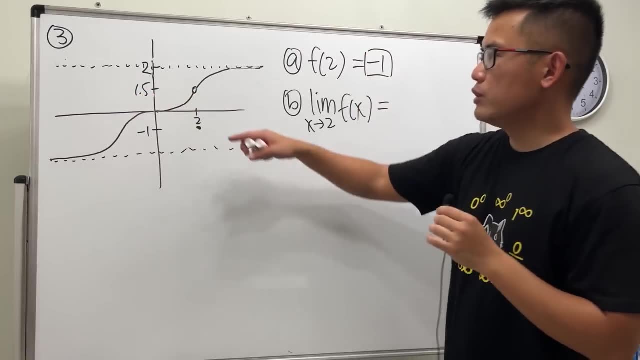 approaching 1.5 when we go from the right and then if we go from the left, the curve is also approaching the wi-fi you 1.5. it's pretty much the y value of this open circle, especially when you have the left and right. 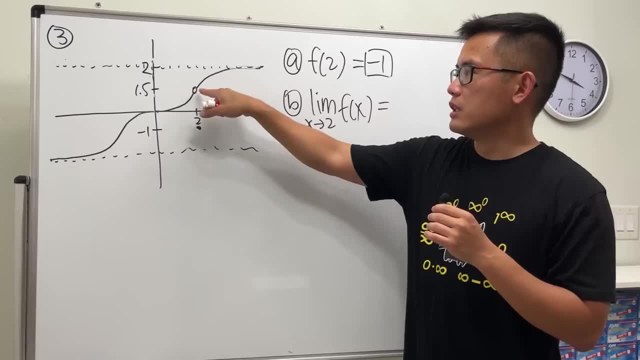 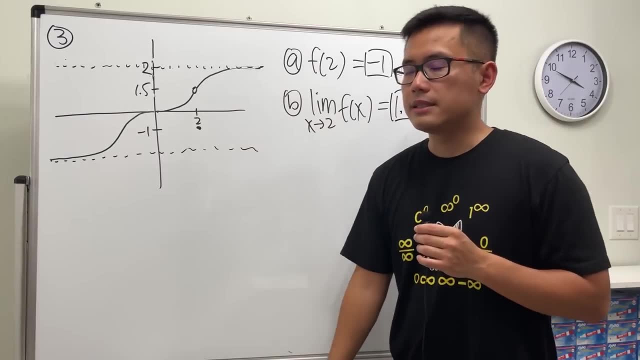 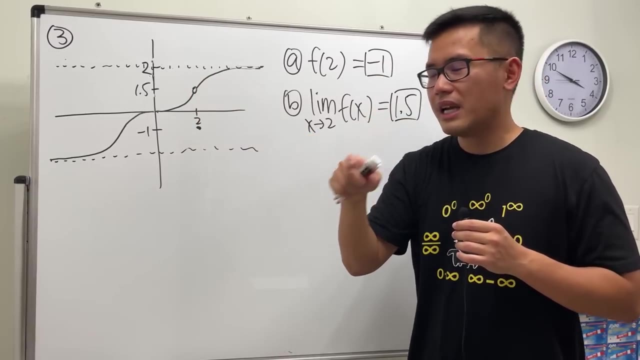 point the left and right end that they're approaching to the same open circle. so it's that 1.5 and in this particular case you see how originally we have a curve, but like we're just missing that, like that little hole right this right here is actually called the removable. 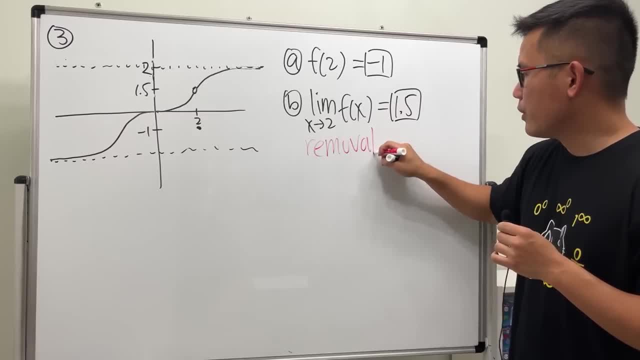 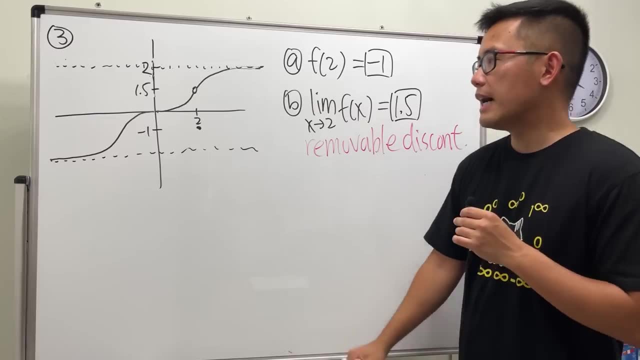 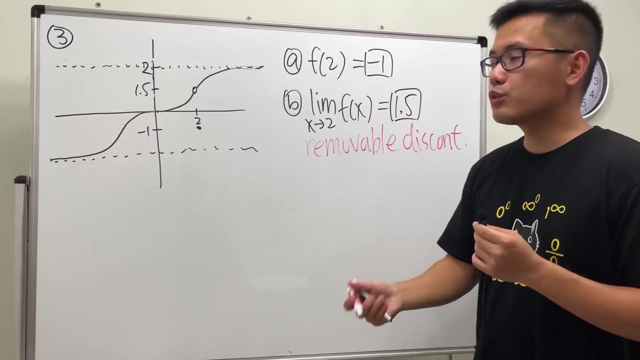 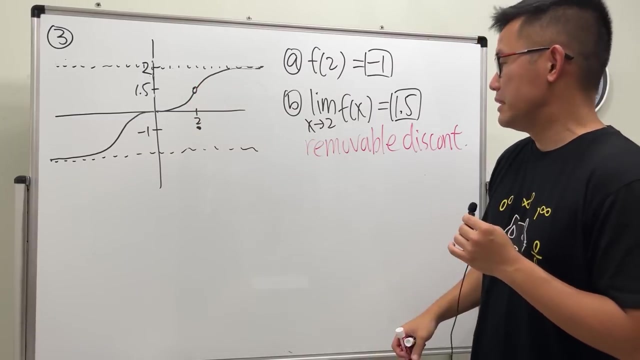 discontinuity. so removable. removable, this continuity, and the reason that is removable. it means that imagine if you just fill in the open circle, guess what? the curve right here will be continuous. that's why you can remove it, meaning that because you can just fix it easily, you can fill in the circle and then no more. this 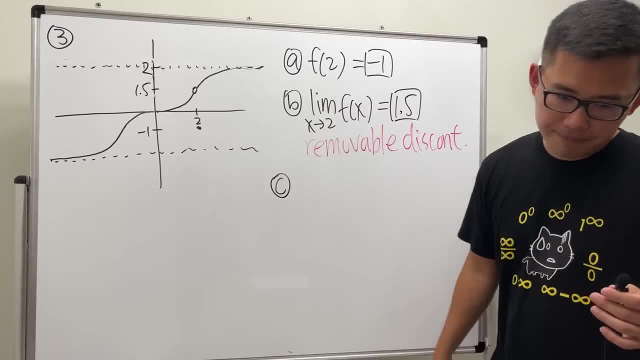 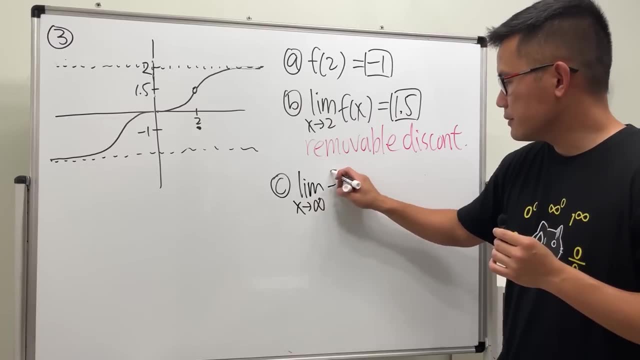 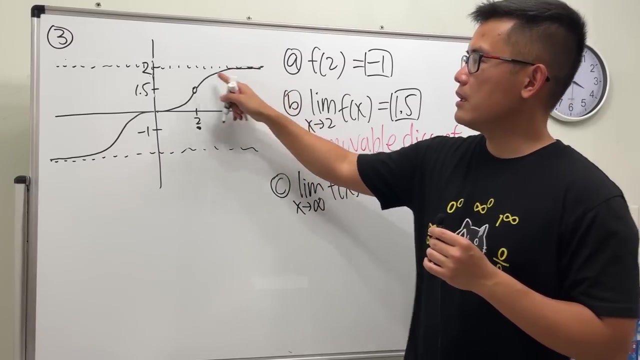 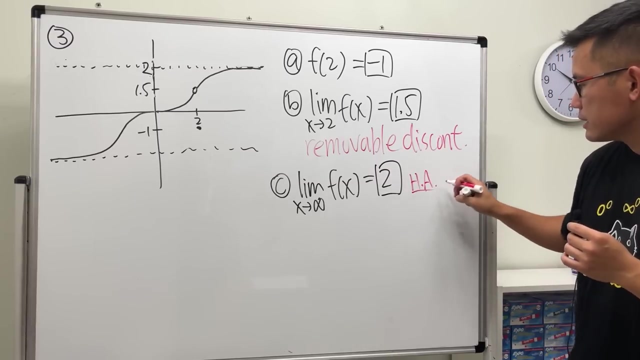 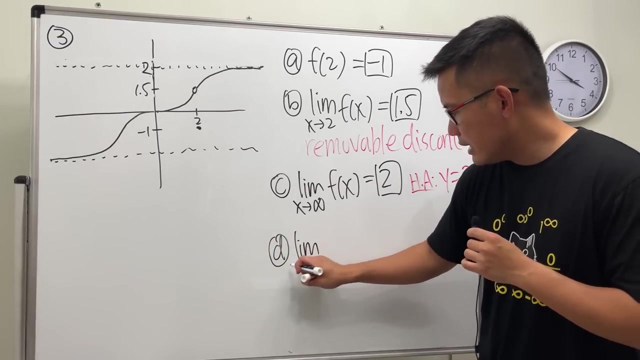 continuous business, all right. number three: limit x approaching infinity. up, up, up, up, up up. and we have a horizontal. stop. here y is 2, right, so is 2, and again here it tells us horizontal, as though y equals 2.. and then, last question: limit as x approaching negative infinity. 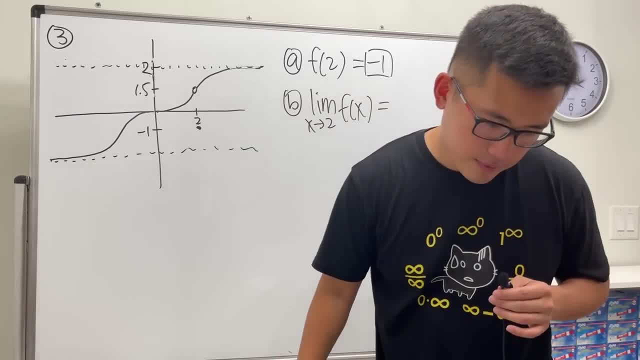 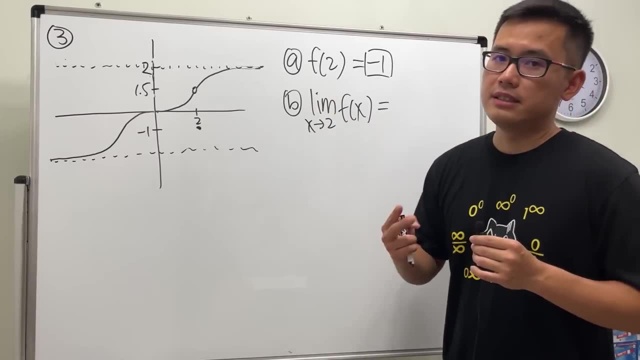 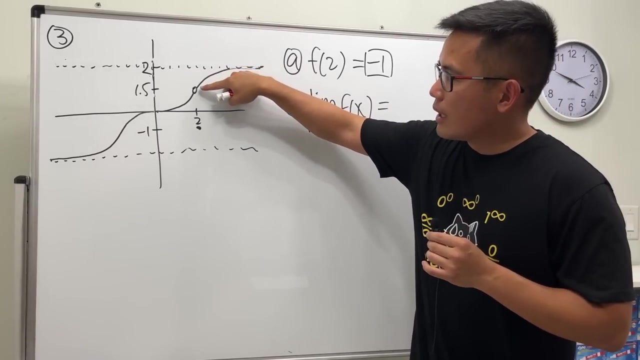 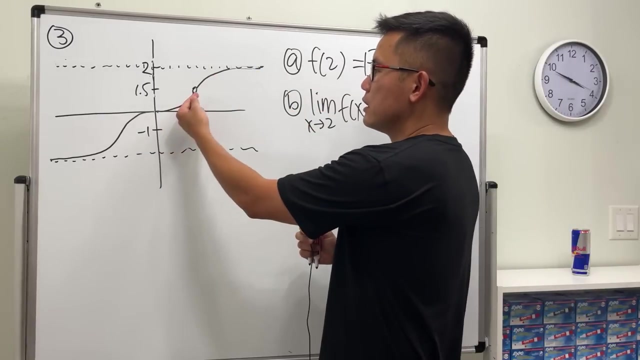 of the function f of x. yeah well, limit as x approaching two. we do not care when x is exactly two, right? so the answer is actually not negative one, but rather you see how the curve is approaching, what. the y file is approaching 1.5 when we go from the right, and then, if we go from the left, the curve is also approaching the y value. 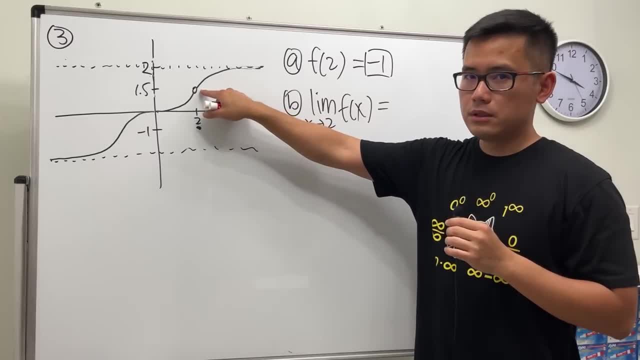 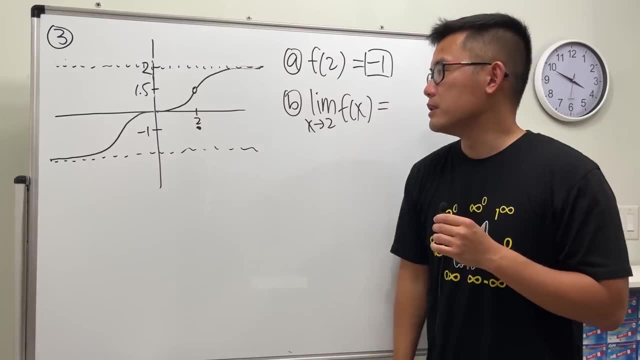 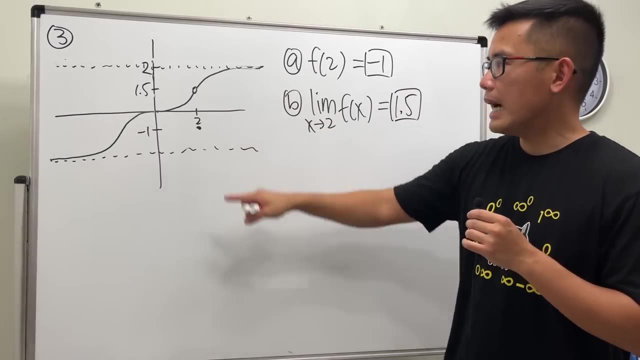 1.5. it's pretty much the y value of this open circle, especially when you have the left and right point, the left and right end, that they're approaching to the same open circle. so it's that 1.5 and in this particular case you see how originally we have a curve, but like we're just 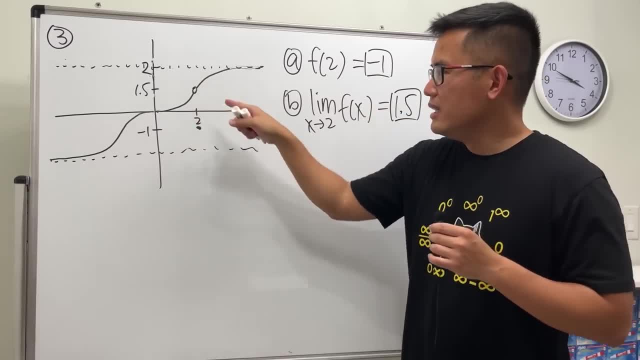 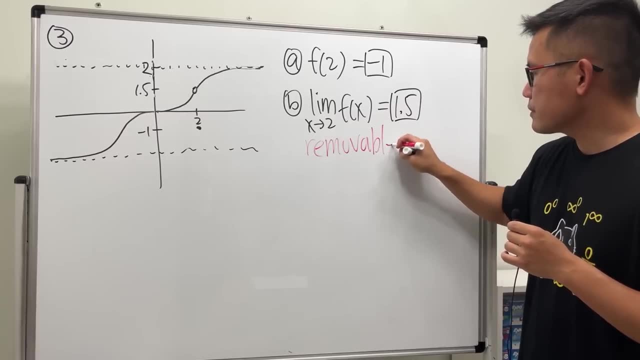 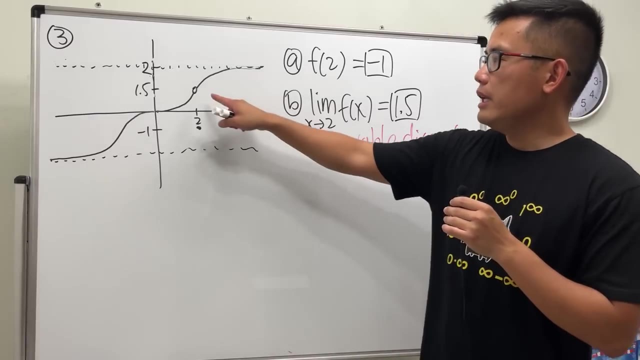 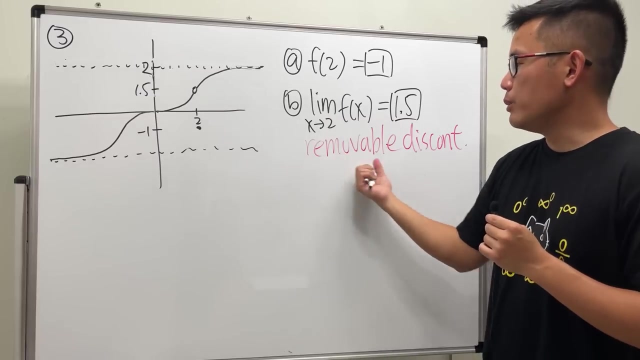 missing that, like that little hole right this right here is actually called the removable discontinuity. so removable, removable discontinuity, and the reason that is removable: it means that imagine if you just fill in the open circle, guess what? the curve right here will be continuous. that's why you can remove it, meaning that because you can just fix it easily. 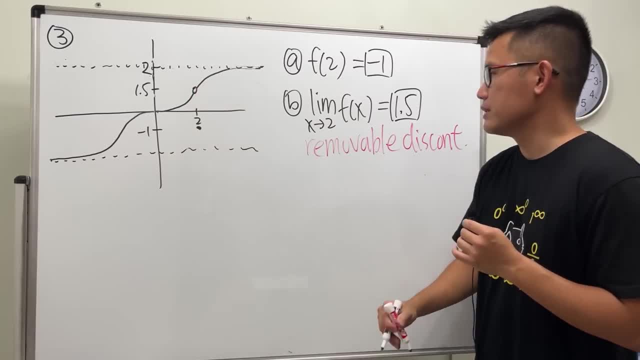 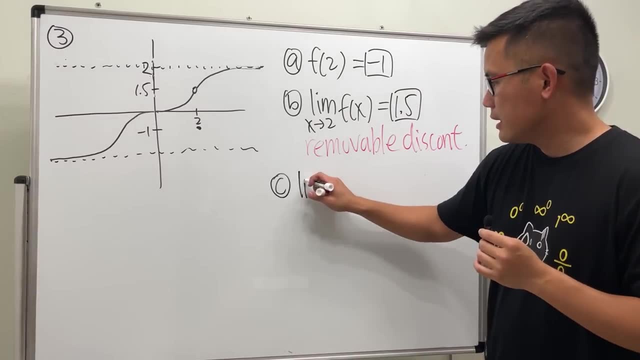 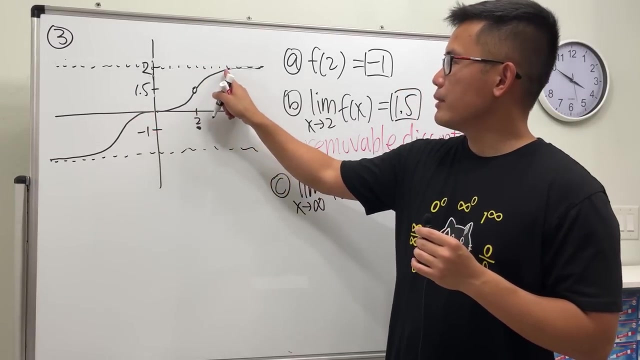 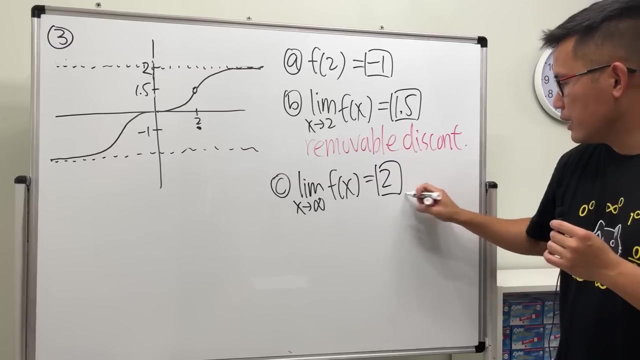 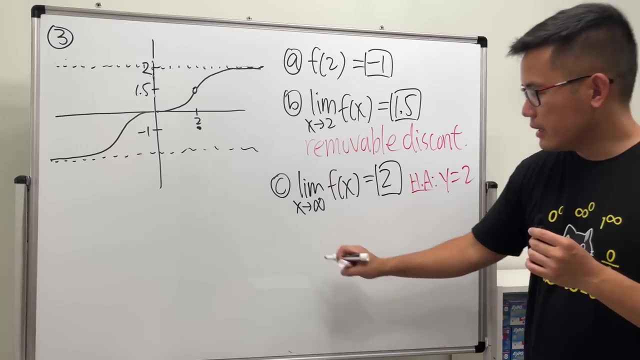 you can fill in the circle and then no more discontinuous business. all right. number three: limit x approaching infinity up. and we have a horizontal stop here y is two, right, so it's two. and again here it tells us horizontal, as though y equals two. and then last question: limit as x approaching negative infinity. 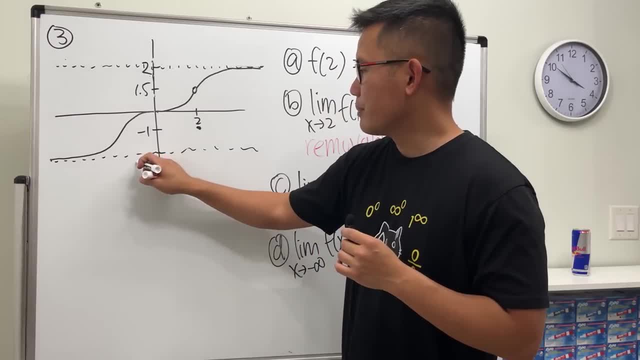 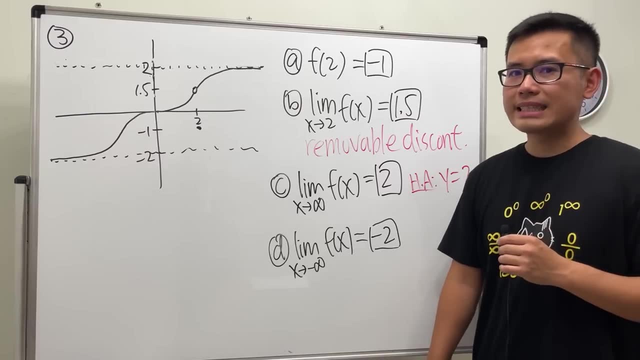 all the way to the left and the y, for here you can look at the picture on the file. it's approaching negative two. and guess what if the question is asking us to find the horizontal isotopes? in fact, we will have two horizontal isotopes. this is the first one. 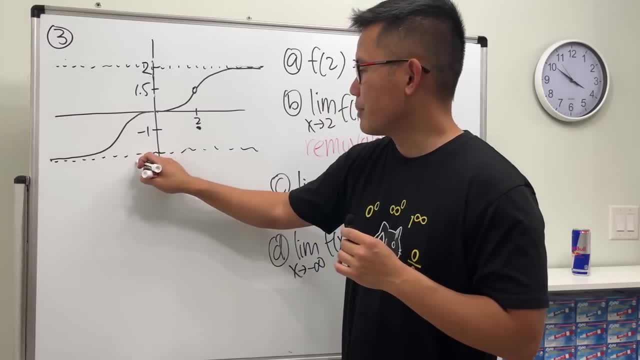 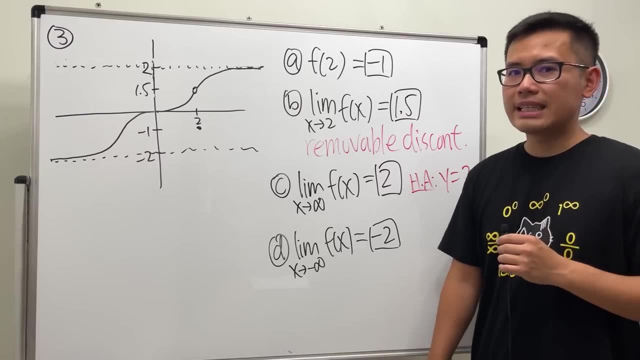 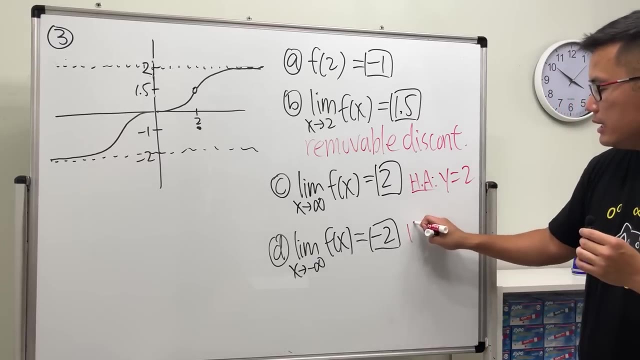 all the way to the left and the y, for here you can look at the picture on the file: it's approaching negative 2.. and guess what? if the question is asking us to find the horizontal isotopes, in fact we will have two horizontal isotopes. this is the first one and the other one is y equals negative 2.. the truth is: 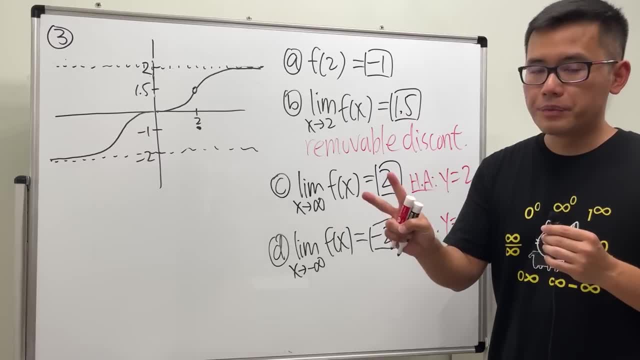 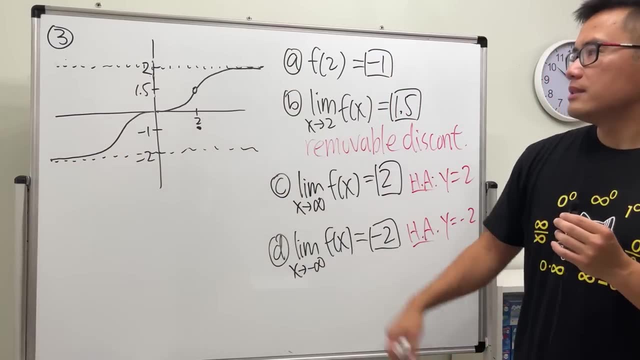 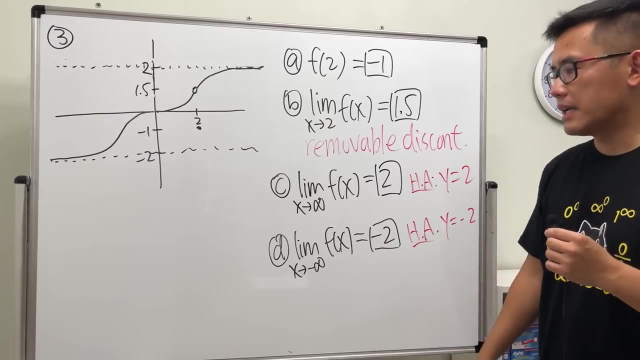 when we have a function, it can have at most two horizontal isotopes. in this case, you can see that we have one here and one there. you may see that this picture is just that we just graph it randomly, right, but in fact inverse tangent also has two horizontal acetone, and you might be wondering. 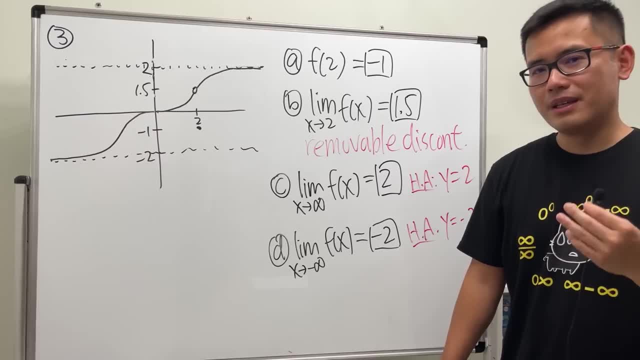 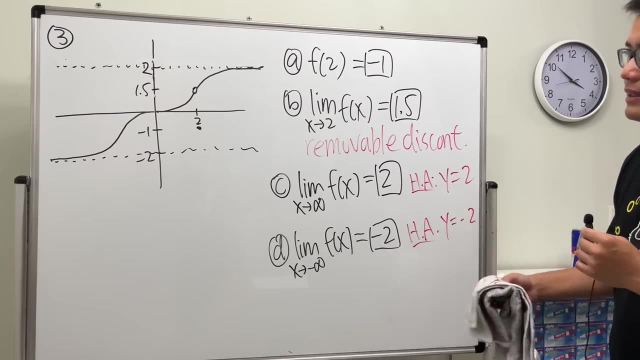 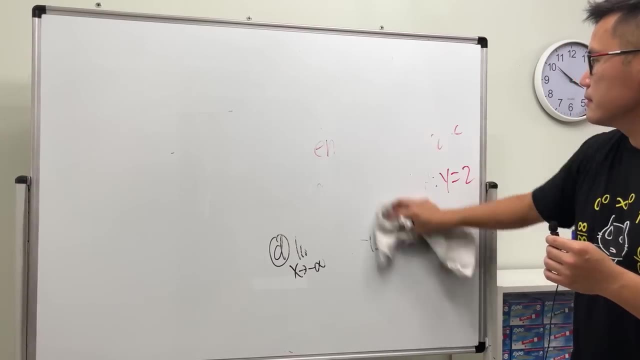 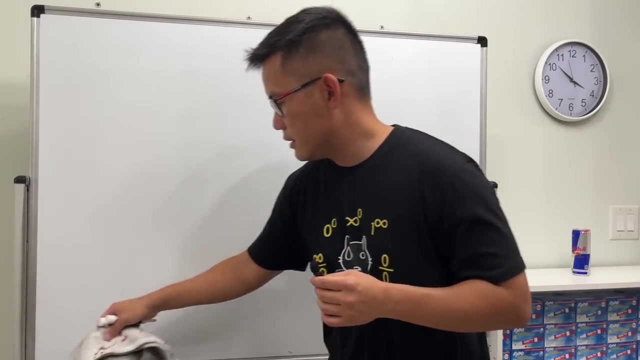 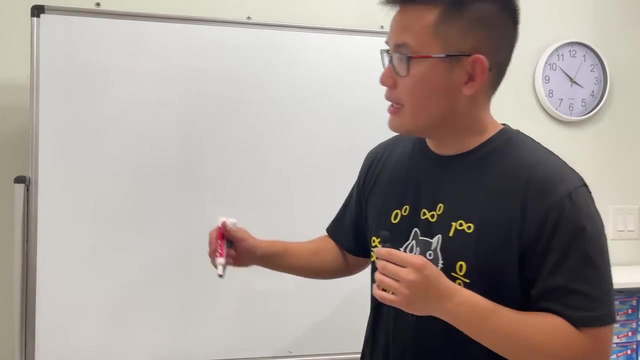 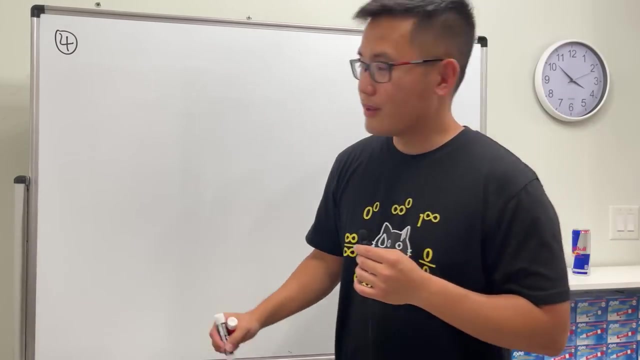 how many vertical isotopes that we have? infinitely many, because if you look at tangent x, it does have infinitely many vertical acetone, by the way. that's it for this right here. so if you look at the first row of the y-axis and you can see that this is the same position, 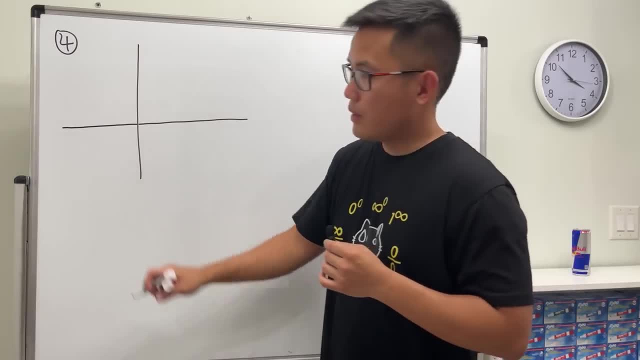 and then you can see that this is the vertical one, that's the horizontal one, this is the vertical one. okay, all right. number four: it's a funny looking picture, kind of it's pretty, though. okay, okay, like this. okay, and then the y for here is 2.. 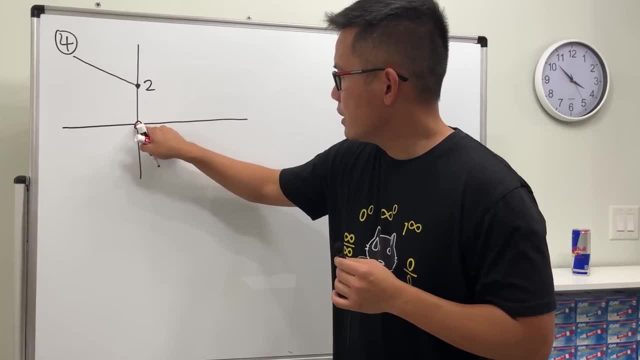 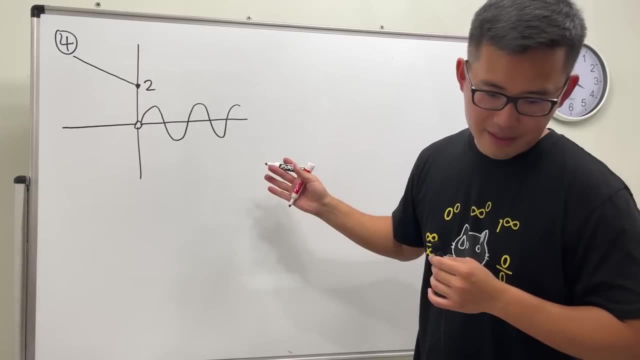 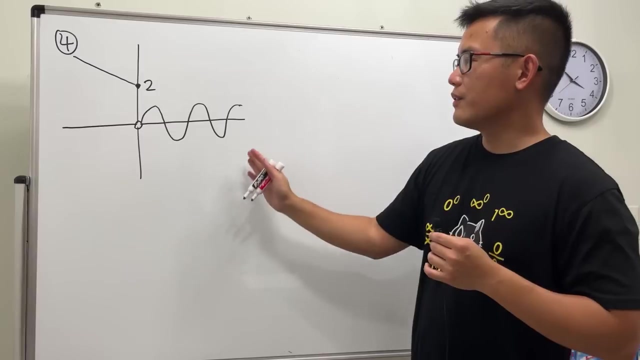 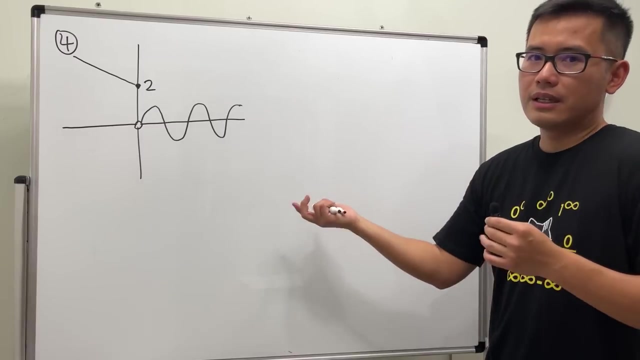 and then open circle here and then we have a wave: okay, someone like this, yeah, and then just kind of continue like this. so here's the deal: whenever you are given like a picture like this, just kind of follow along. what's the trend of the curve? in this case, it continues. it's like a sine or cosine. it's more like a. 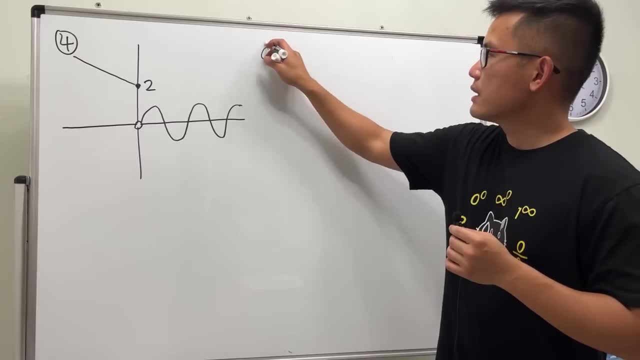 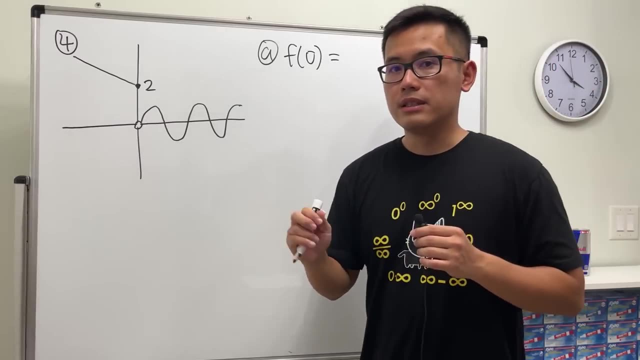 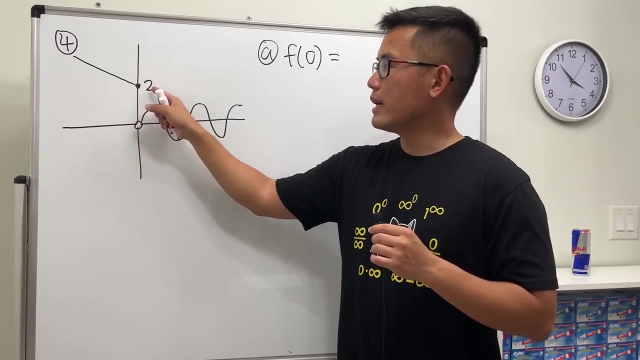 sine curve because it starts with zero. right here, right, okay, part a, let's find the value for f of 0. this means when X is exactly 0, right, X value exactly 0. we look at a closed circle. go up here. the Y is 2, so the answer here is 2. done, yay. 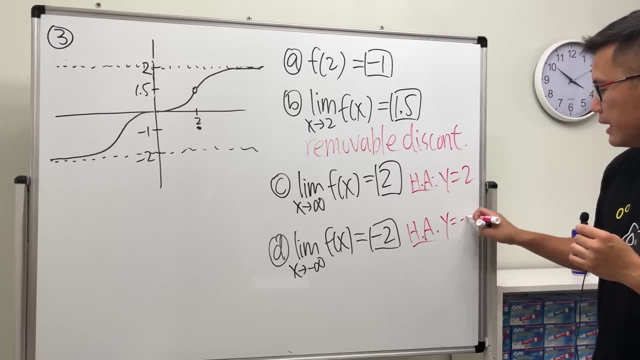 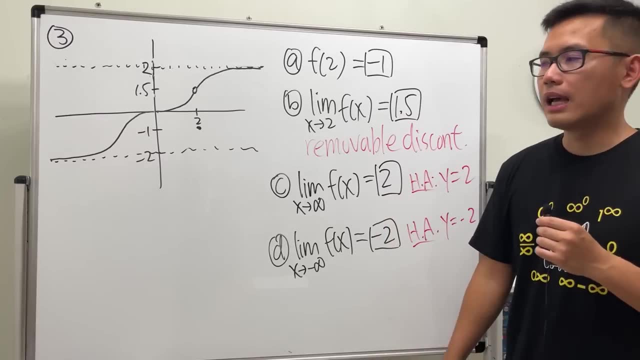 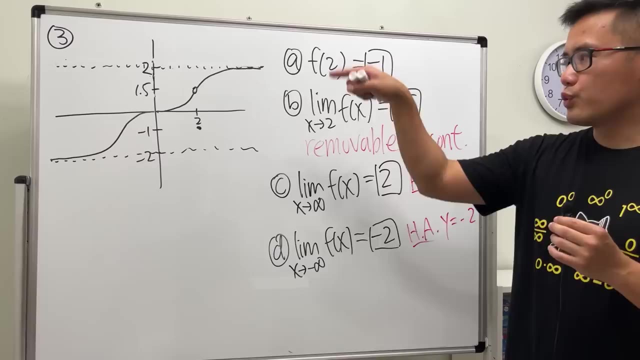 and the other one is y equals negative two. the truth is, when we have a function, you can have at most two horizontal isotopes. in this case, you can see that we have one here and one here. you may think that, hey, this picture is just that we just graph it randomly, right? but in fact in the 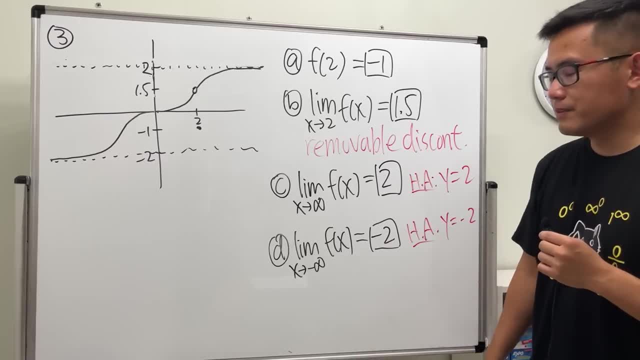 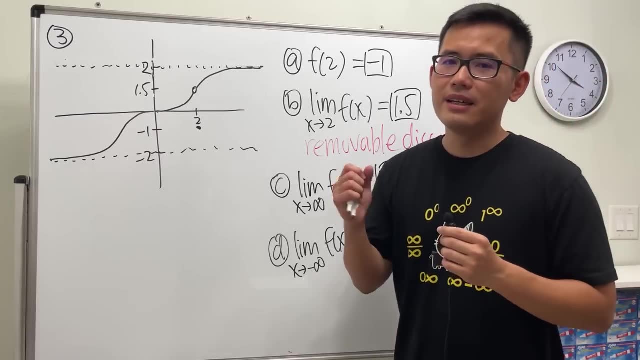 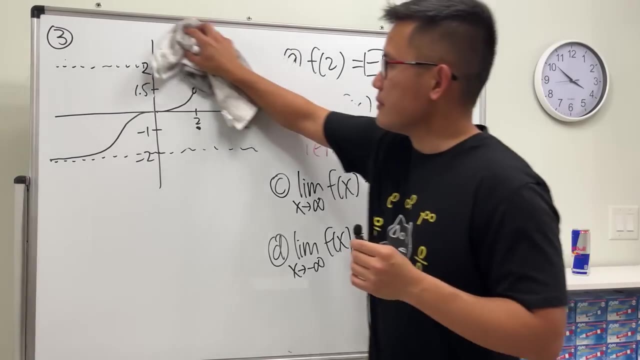 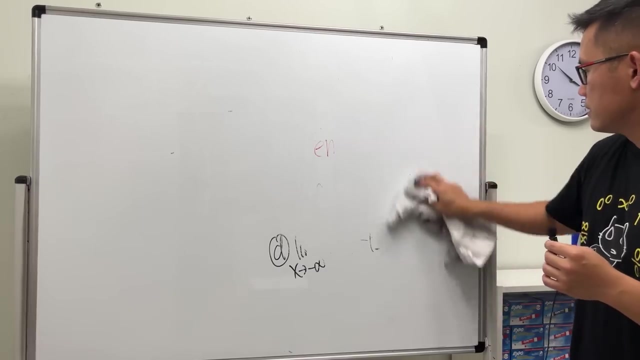 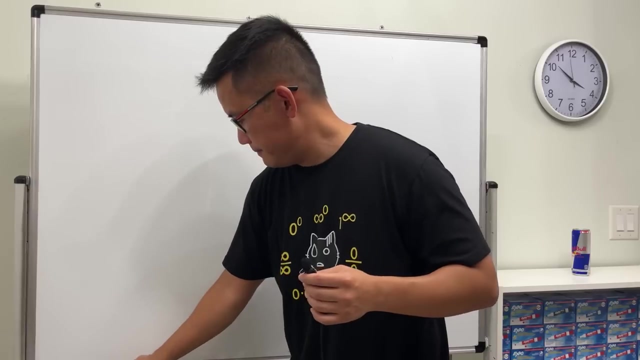 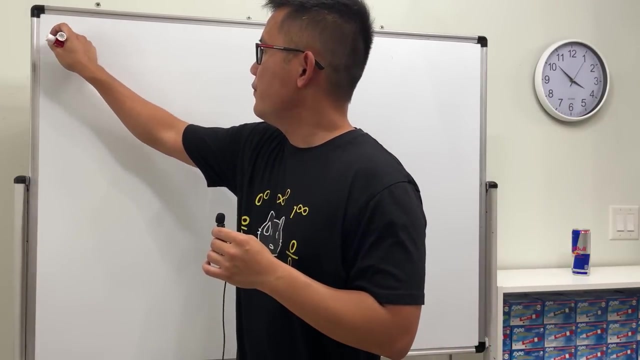 first tangent also has two horizontal isotope, and you might be wondering how many vertical isotopes that we have. infinitely many, because if you look at tangent X, it does have infinitely many vertical isotope. by the way, that's it for this, right here. all right, number four: it's a funny-looking picture, kind of it's. 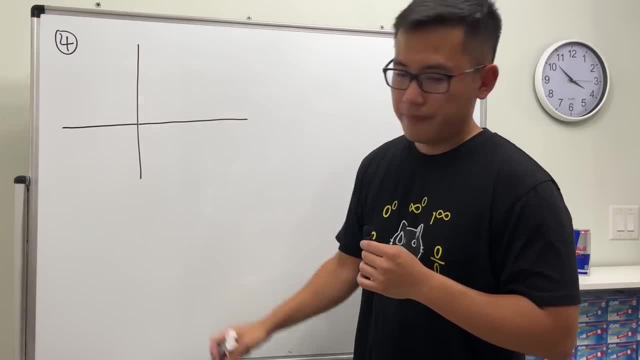 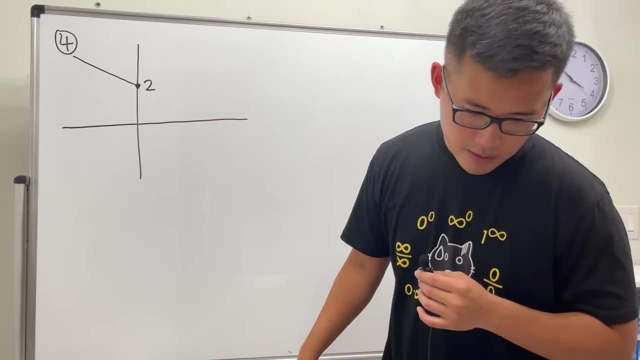 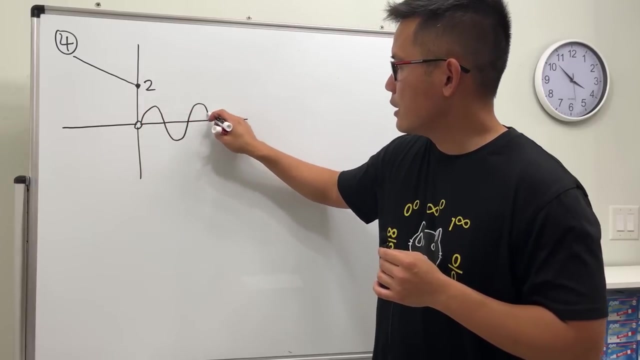 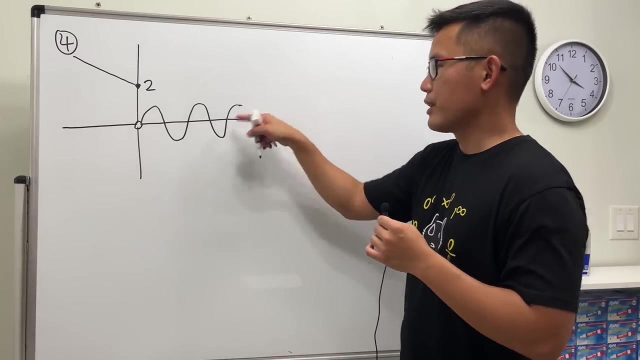 pretty, though, okay, okay, okay, yes, okay, and then the Y bar here is two, then open circle here, and then we have L, okay, and then the Y bar here is two, and then open circle here, and then we have L wave, okay, someone like this, yeah, and then just kind of continue like this. so here's the deal. whenever you are. 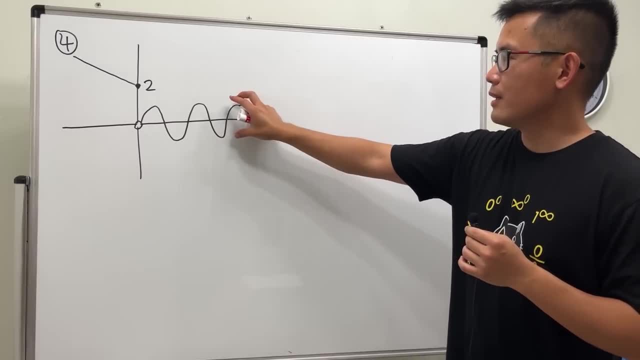 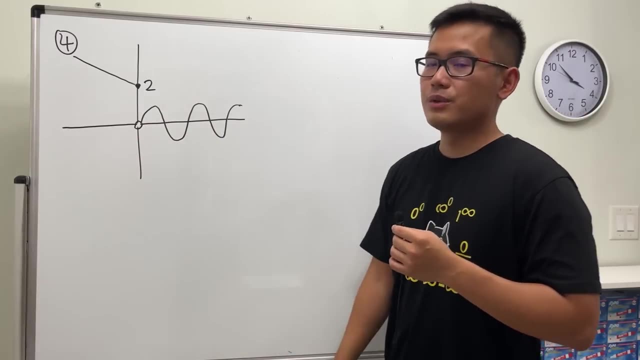 given like a picture like this: uh, just kind of follow along. what's the trend of the curve? in this case, it continues. it's like a sine or cosine. it's more like a sine curve because you start with zero, right here. right, okay, part a, let's find the value for. 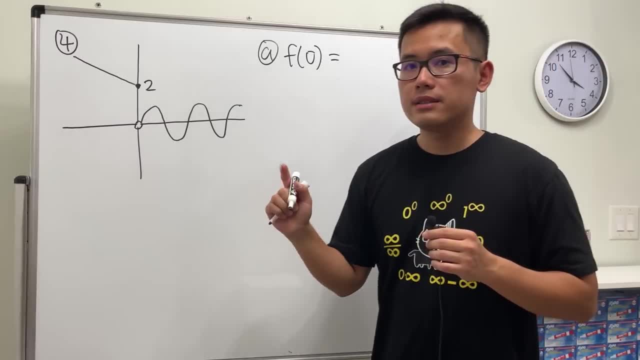 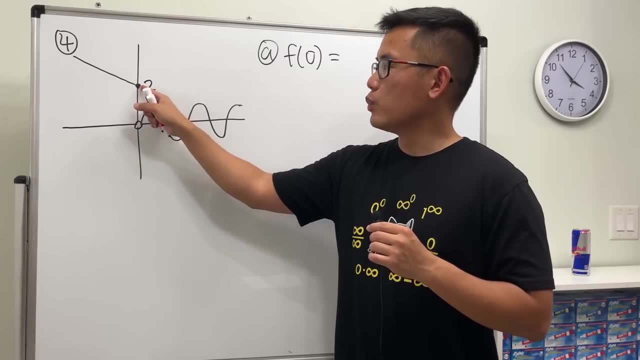 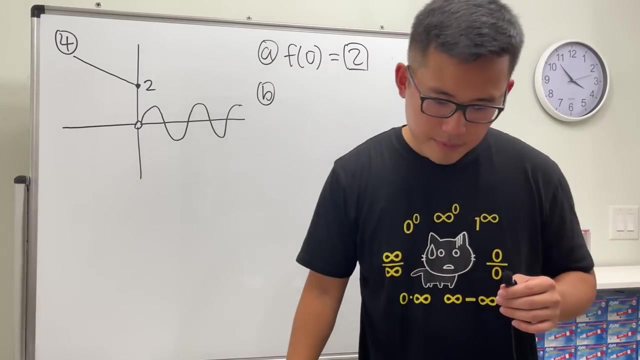 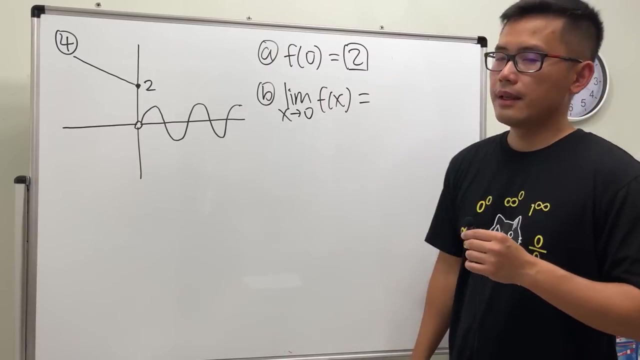 f of zero. this means when x is exactly zero, right, x value, exactly zero. we look at the closed circle. go up here: the y is two, so the answer here is two done, yay, b, the limit as x approaching zero. f of x. what do you guys think? i'll tell you first. 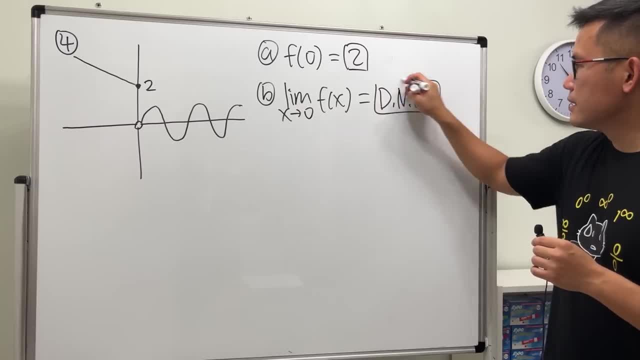 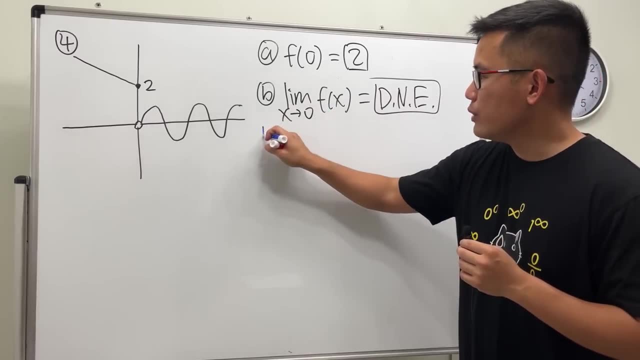 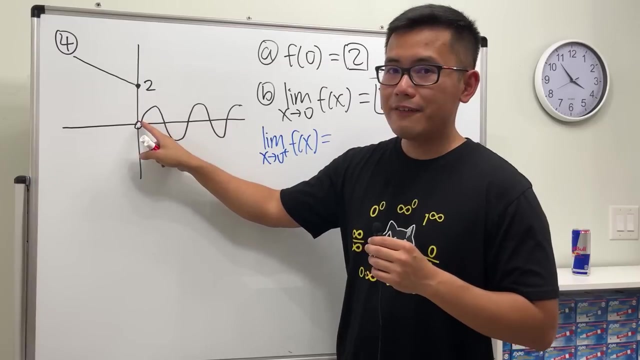 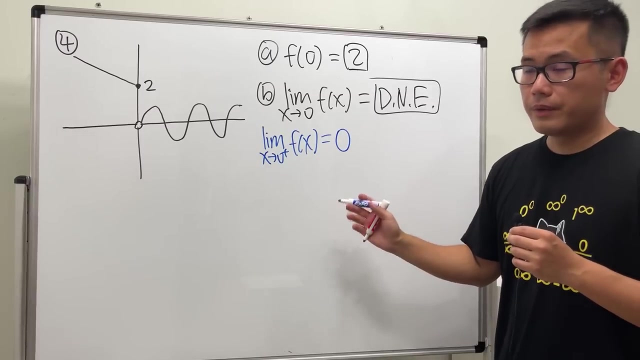 answer does not exist. why? because, again, we do not have the plus or minus, so we actually have to do both. and if we look at the limit as x approaching zero plus, the y value is approaching zero. right, the y value is approaching zero when we go from the right, so this right here is zero. 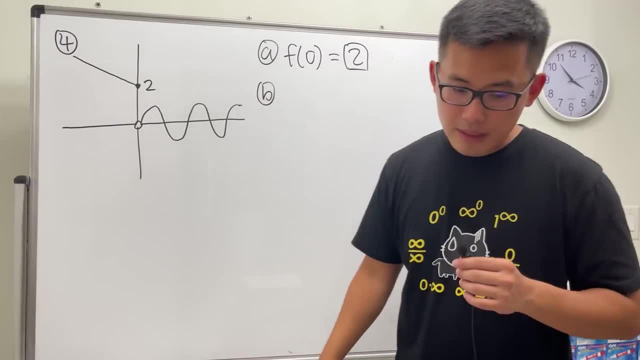 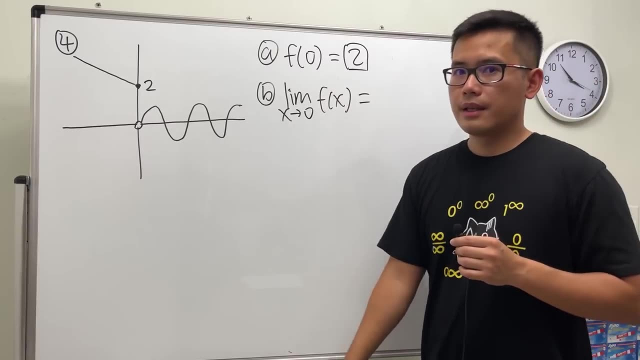 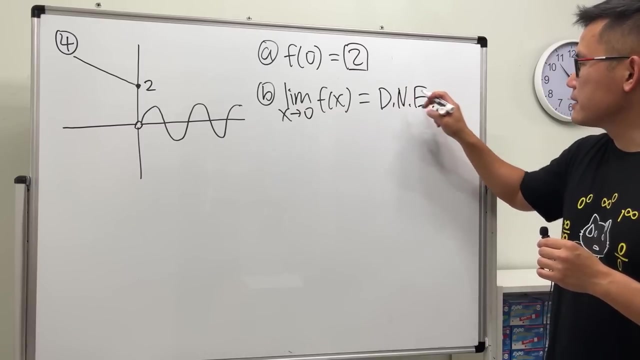 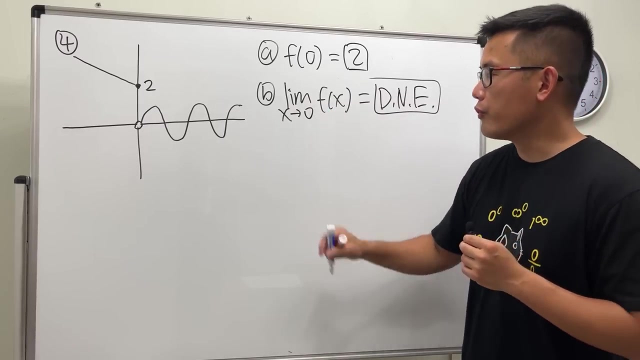 B, the limit as X approaching 0. f of X. okay, so we have a curve like this, and then we have a curve like this, and then we have a. what do you guys think? I'll tell you first answer: does not exist. why? because, again, we do not have the plus or minus, so we actually have to do both. and if we 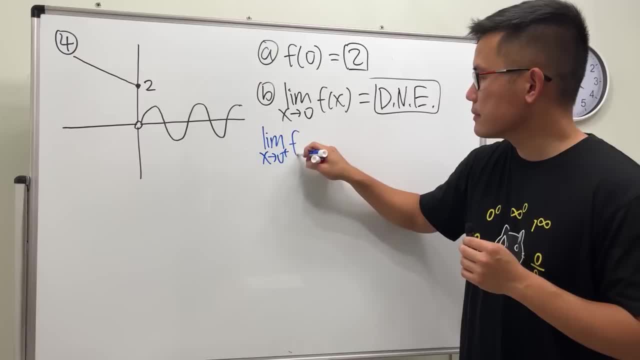 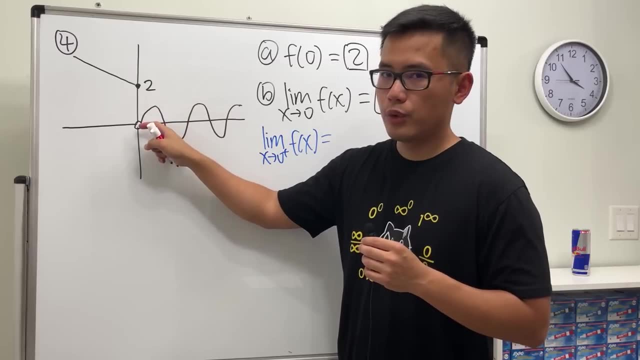 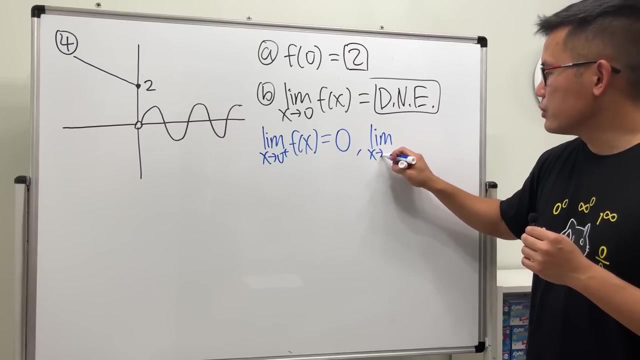 look at the limit as X approaching 0 plus, the Y value is approaching 0. right, that Y value is approaching 0 when we go from the right, so this right here is 0. however, if we look at the limit as X approaching 0 minus, use your left hand. 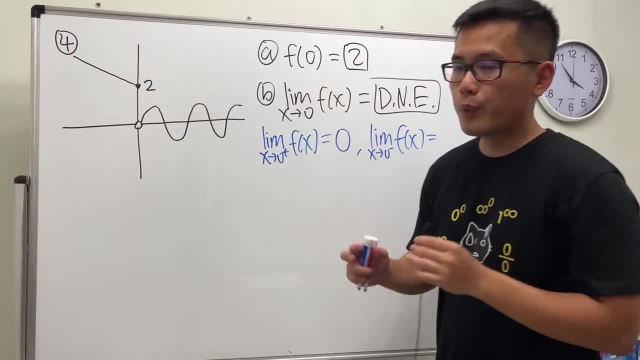 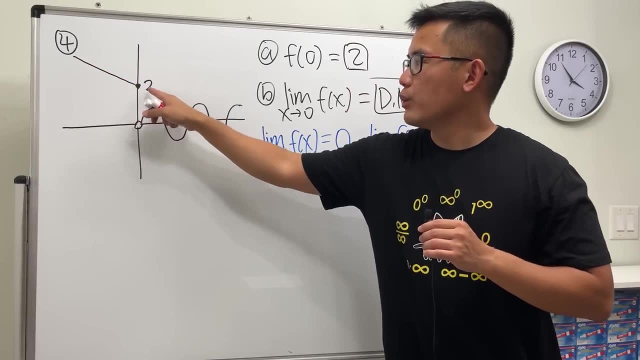 you see, the Y for is approaching 2 and again, when we are talking about the limit, we do not care about when X is exactly 0 approaching and the Y for here is 2. when we go from the left hand side and you see 0 and 2, they are definitely. 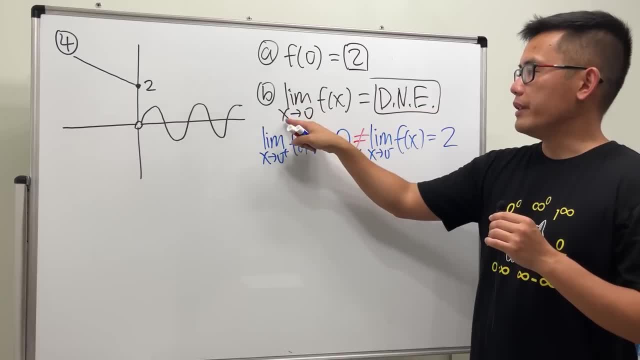 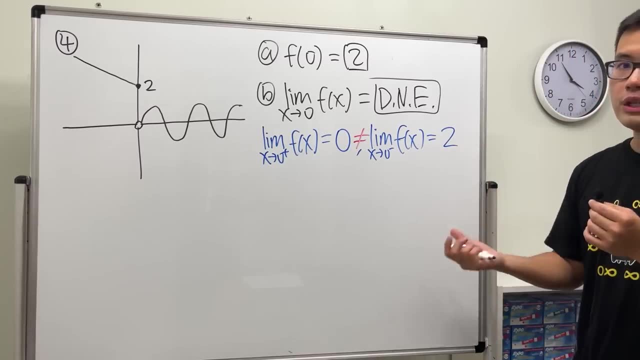 not equal. that's why the limit does not exist when X is approaching 0. that's why the limit does not exist when X is approaching 0- 0. however, though, if this is the question, then this is the answer. if this is the question, that's the answer so you can have. you will have to answer the 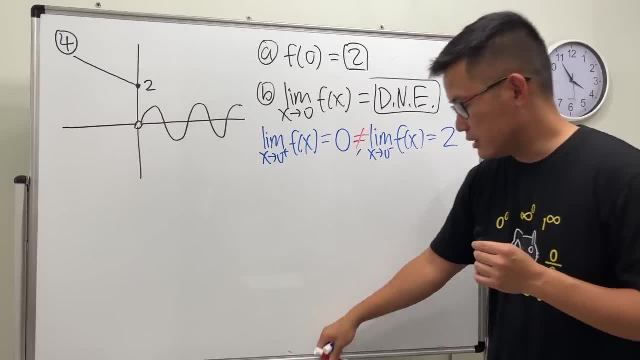 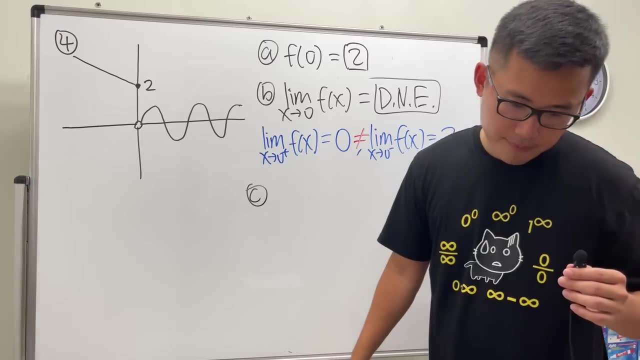 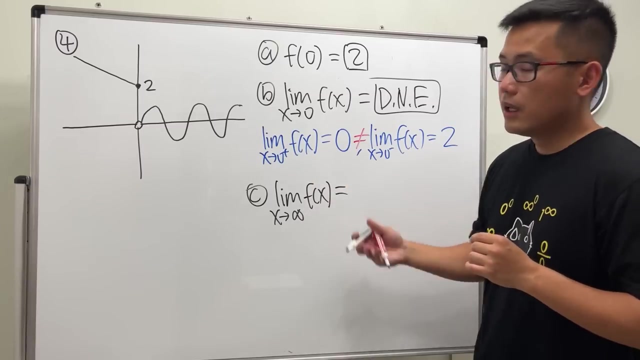 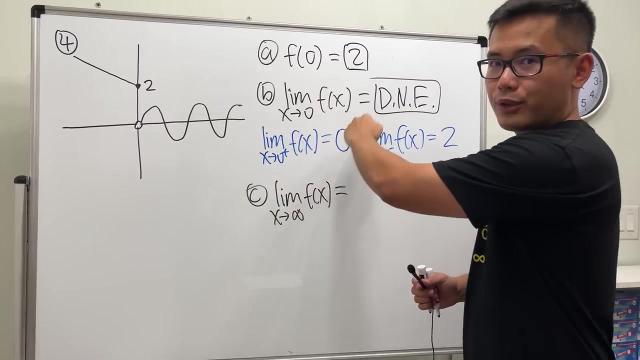 individually. but for this does not exist, is the answer, because the positive and negative in the minus version they do not equal. all right limit as X approaching positive infinity, do we have any horizontal as though? no, because again, If you follow the curve it keeps going up and down, up and down, right. 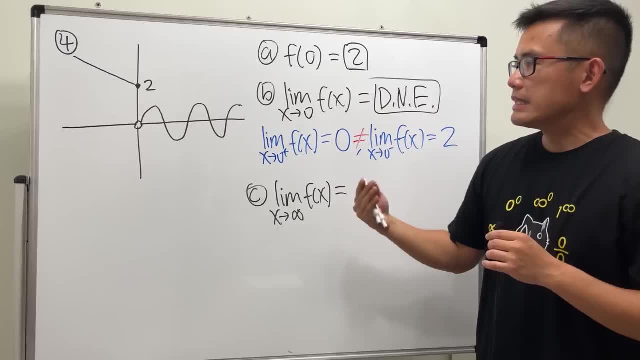 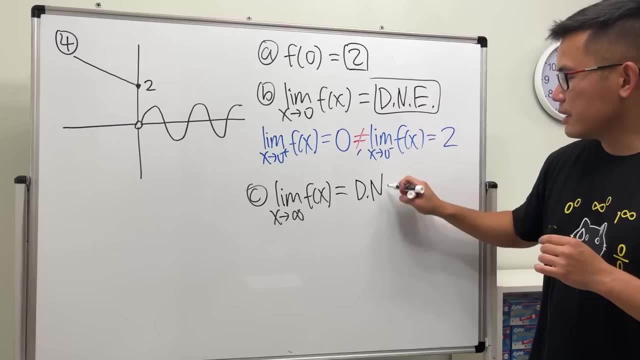 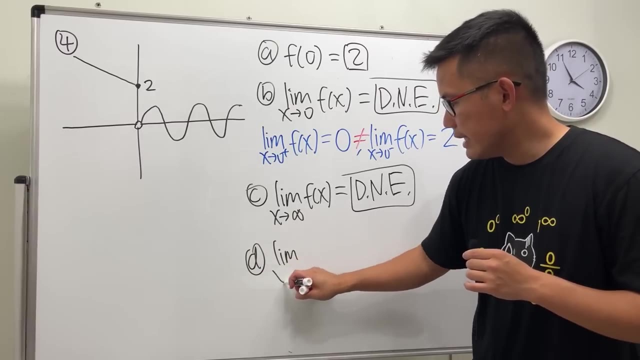 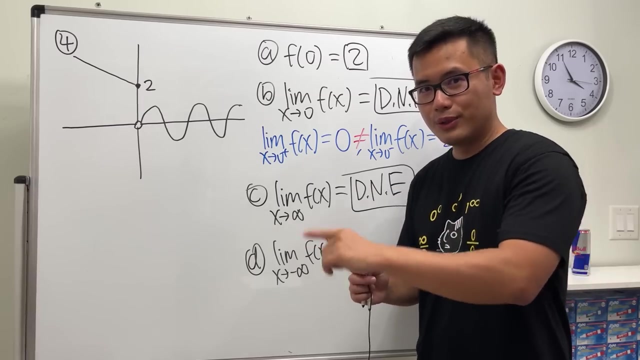 So the value of the function does not approach to y value as x goes to infinity. So here this right, here we also say: doesn't exist, Doesn't exist The limit as x approaching negative infinity, f of x. This means x is approaching to the left all the way, right. 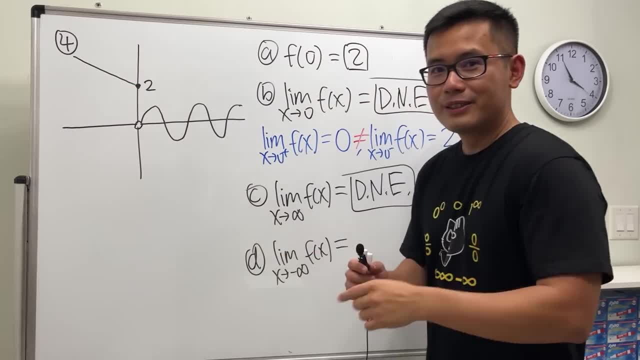 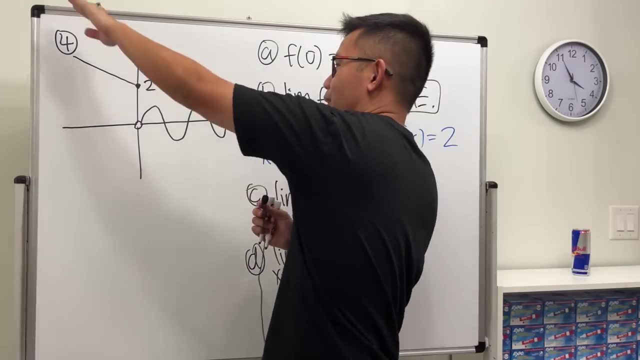 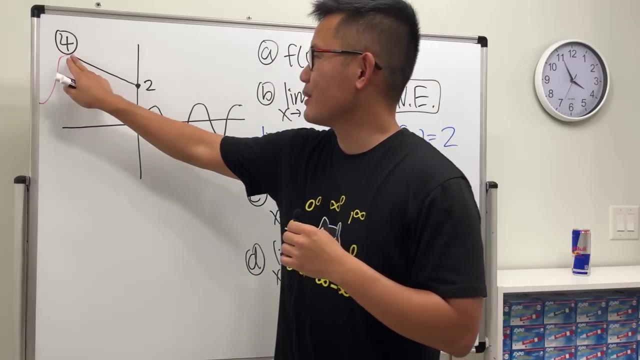 So ready. So again, if this is the picture all the way, that way, then do not just say, hey, it's going to come down. No, no, no, Nobody is going to do that to you, all right. 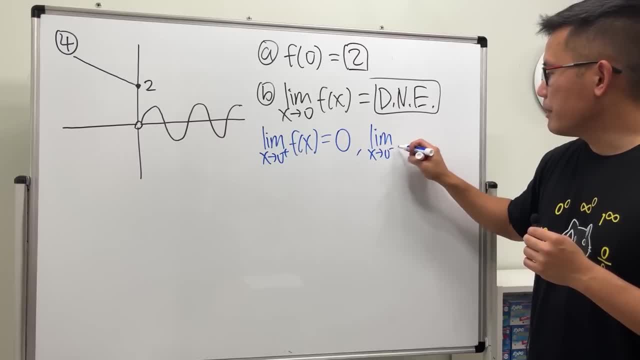 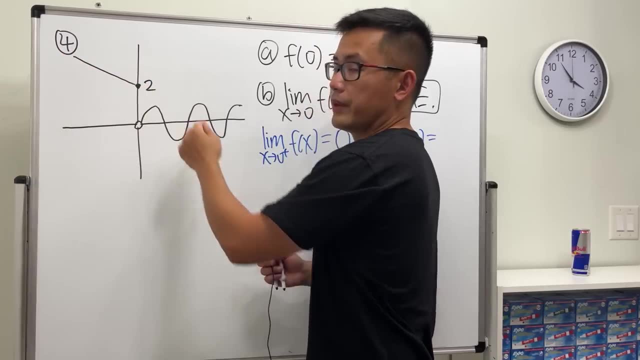 however, if we look at the limit as x approaching zero minus, you see the y value is approaching zero. you use your left hand, you see the y value is approaching two. and again, when we are talking about the limit, we do not care about when x is exactly zero. 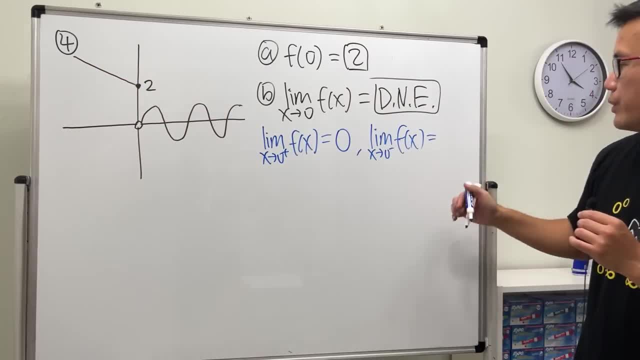 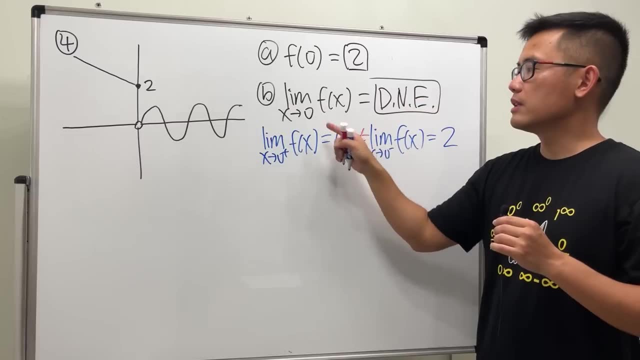 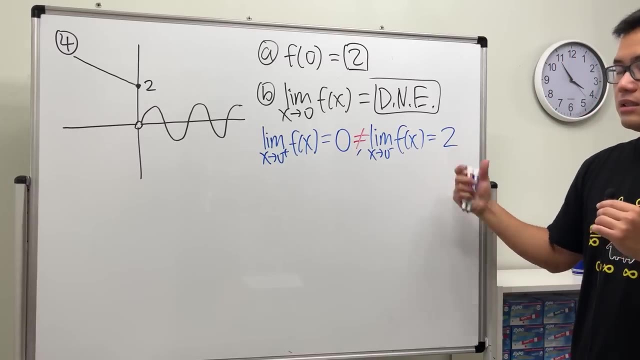 right, you see approaching and the y, for here is two. when we go from the left hand side, and you see zero and two. they are definitely not equal. that's why the limit does not exist when x is approaching zero. however, though, if this is the question, then this is the answer. if this is the question, that's the answer, so you can. 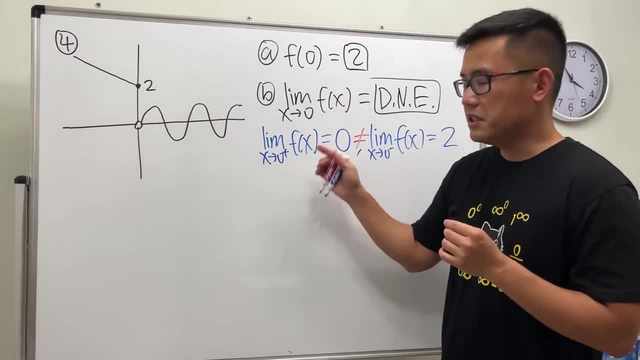 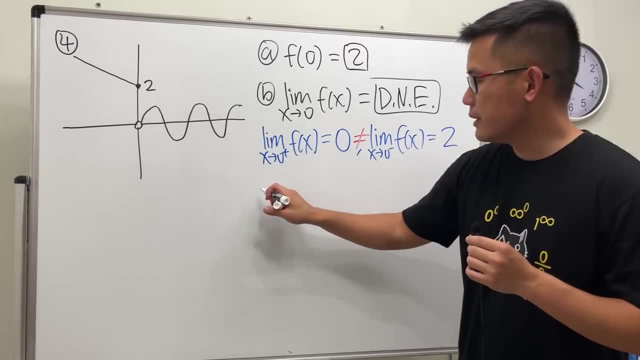 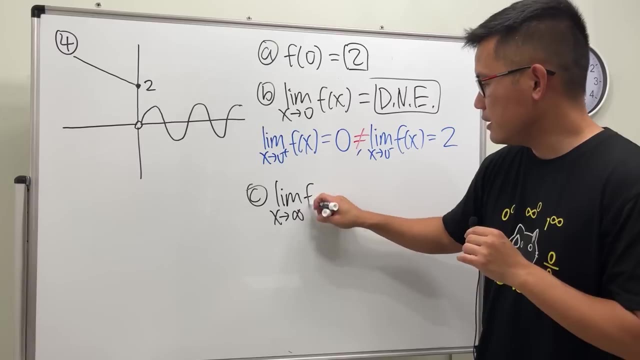 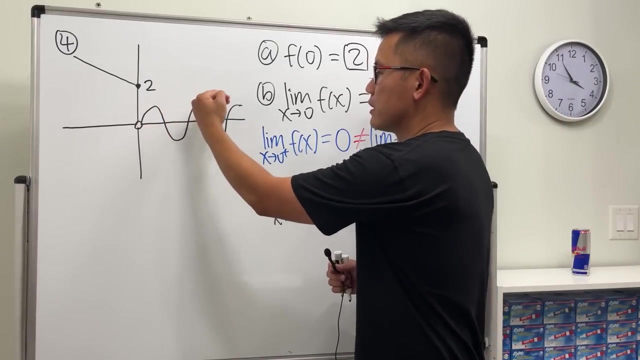 have, you will have to answer that individually, but for this does not exist. is the answer? because the positive and the negative in the minus version they do not equal. all right limit as x approaching positive infinity, do we have any horizontal as though? no, because again, if you follow the curve it keeps going up and down, up and down, right. 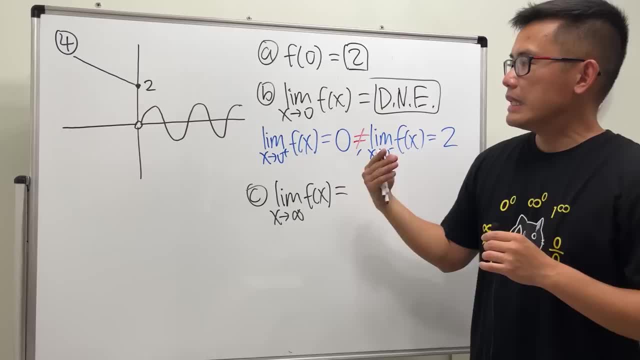 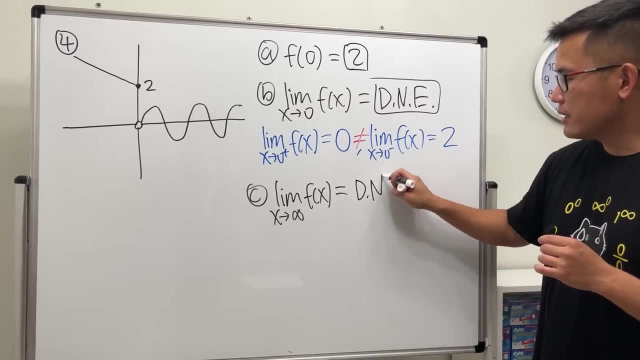 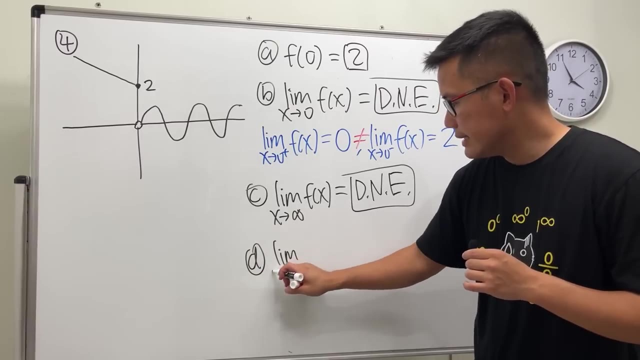 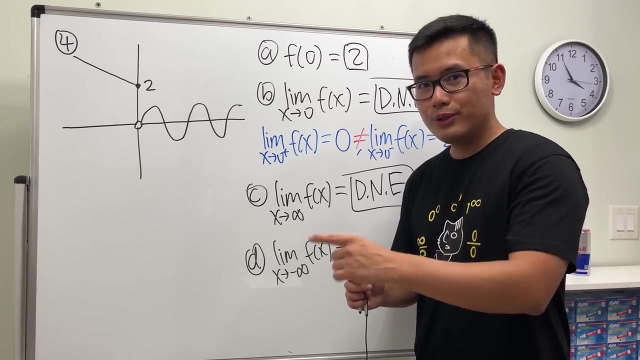 so the value of the function does not approach to a y value as x goes to infinity. so here this right. here we also say: doesn't exist, doesn't exist. d limit as x approaching negative infinity. f of x. this means x is up approaching to the left all the way right, so ready. 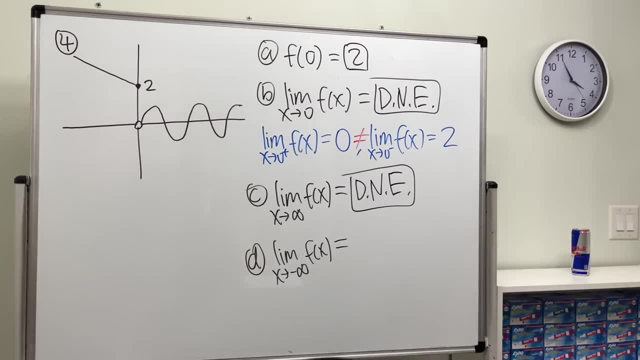 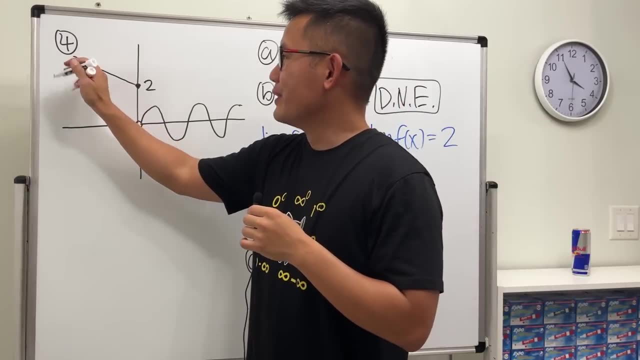 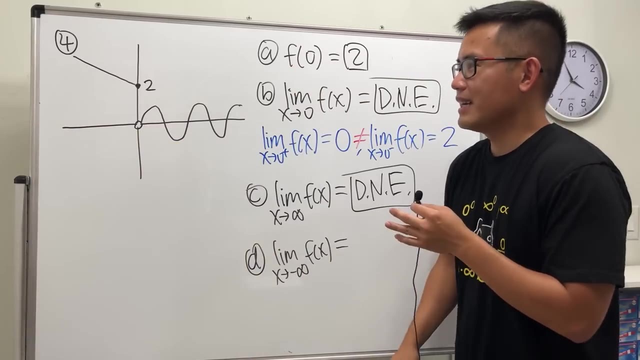 so again, if this is the picture, then all the way, all the way. that way, then, uh, do not just say, hey, it's going to come down, no, no, no, nobody is going to do that to you all, right, if a test is like that, then people will be upset, but anyway though, yeah, that's the case. 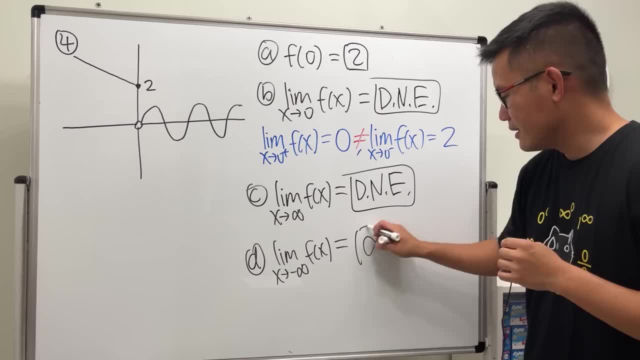 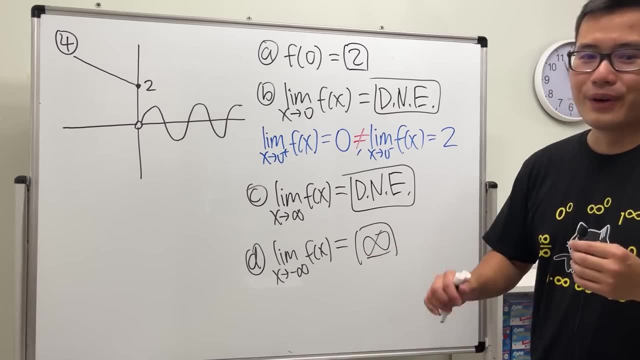 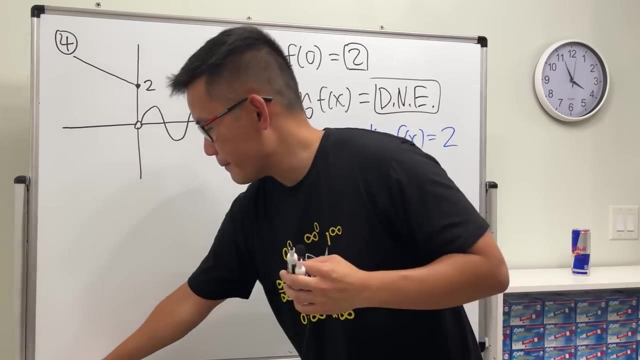 so the answer is past the infinity, because the wi-fi is all the way out, all the way up. so this is d, and then this is the number four, first page done, cool, huh, but i know it's just a lot of graphs. that's why, and i know, i dropped the microphone, hopefully. 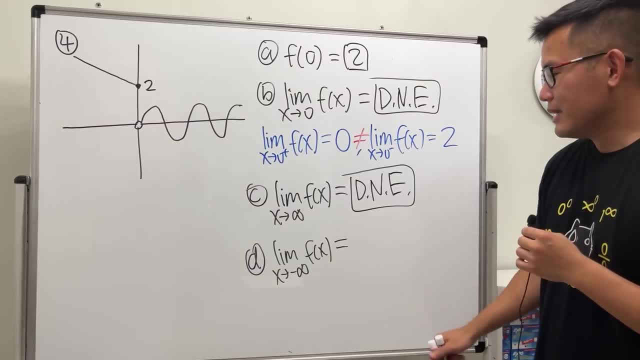 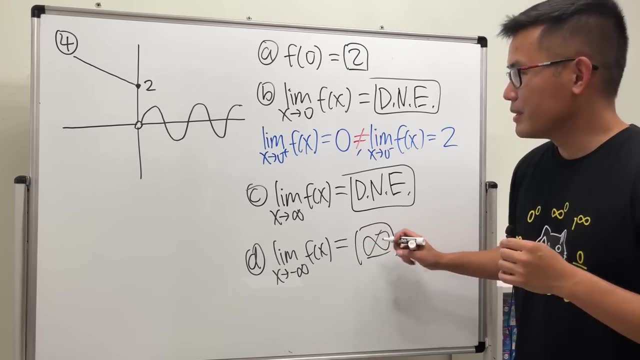 If a test is like that, then people will be upset, But anyway, yeah, That's the case. So the answer is positive: infinity, Because the Wi-Fi is all the way out, all the way out. So this is D, and then this is number four. 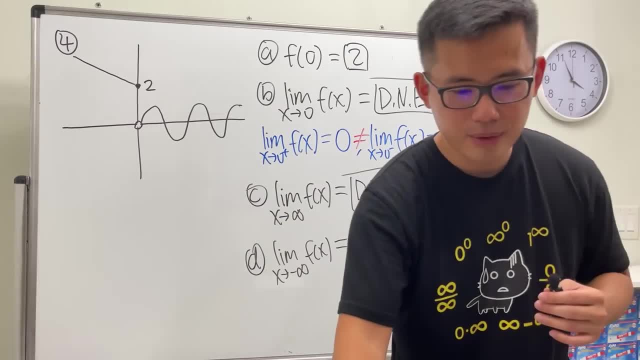 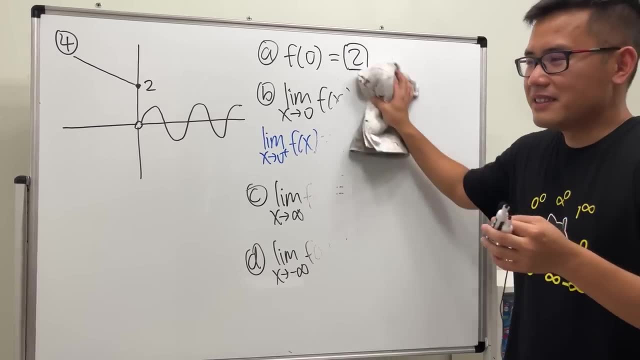 First page done, Cool huh, But I know it's just a lot of graphs. That's why- And I know- I dropped the microphone. Hopefully it's okay, Because in fact this is my new microphone, Because the previous microphone 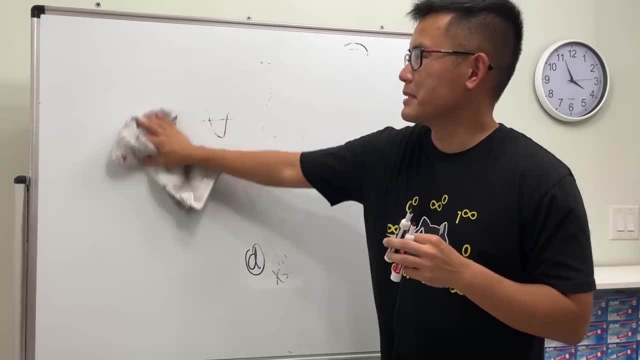 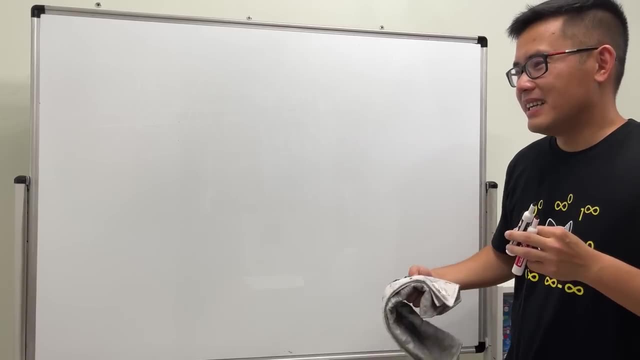 Yeah, I don't know. I don't know what happened, but it just got bad And I'm pretty sure it's because I dropped a lot. Not a lot, but I dropped a few times. Yeah, let me just use that. 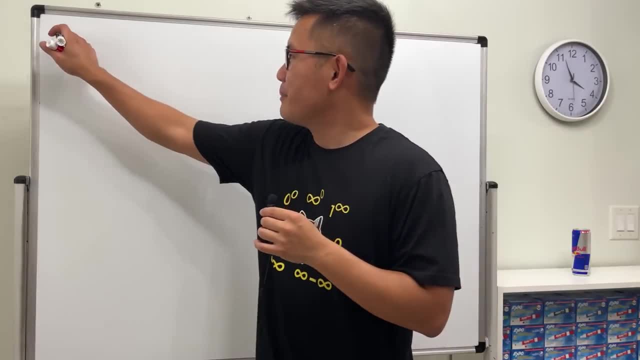 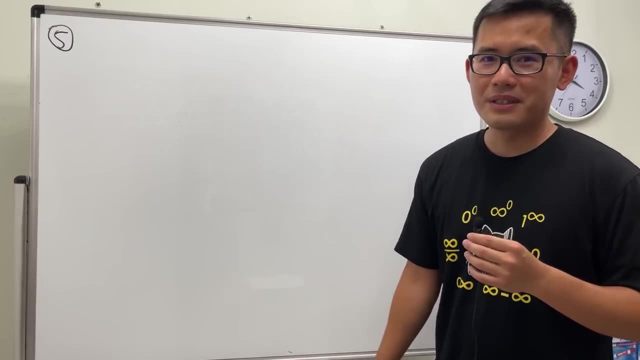 I don't know how many is a lot, But anyway, number five, Number five. If, because I dropped it earlier and then the sound went back and then I broke it, that would suck, Because I cannot hear how the sound is recorded right now. 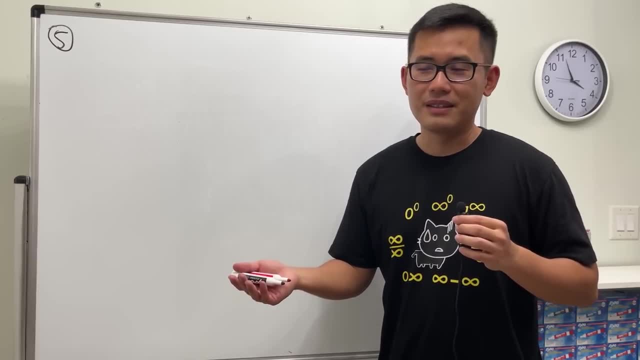 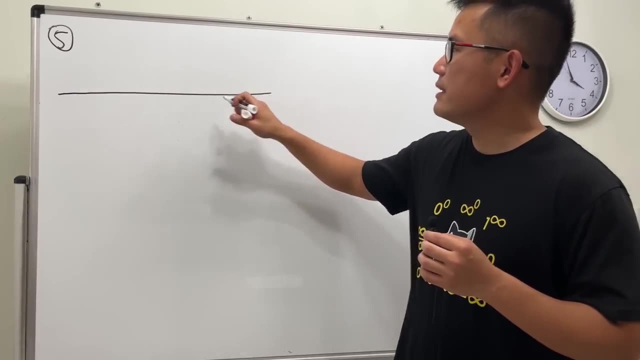 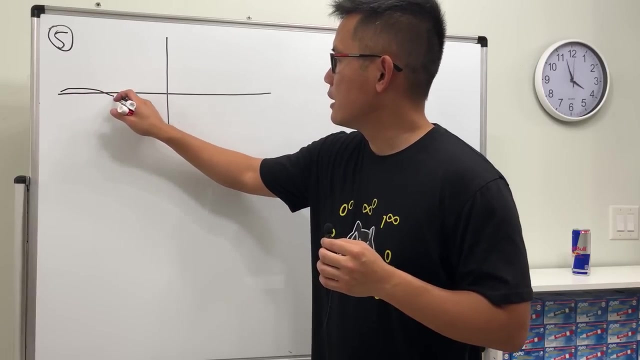 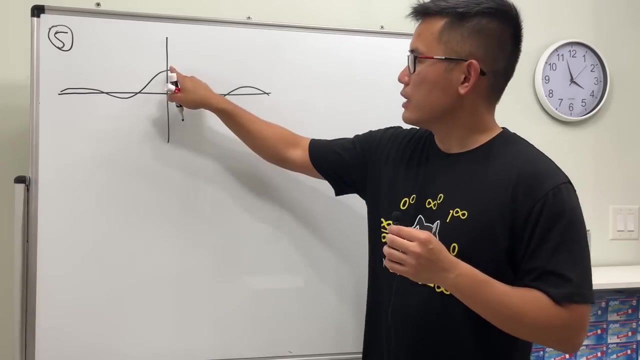 This is question number five on the 96 questions to go. Anyway, All right, Number five. this is the famous question right. So the curve looks like this, Something like that right, And in fact here we have an open circle. 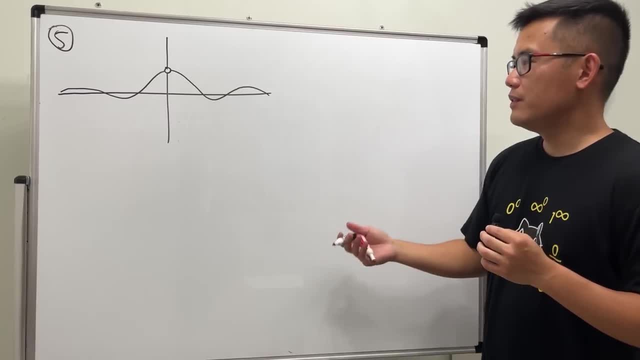 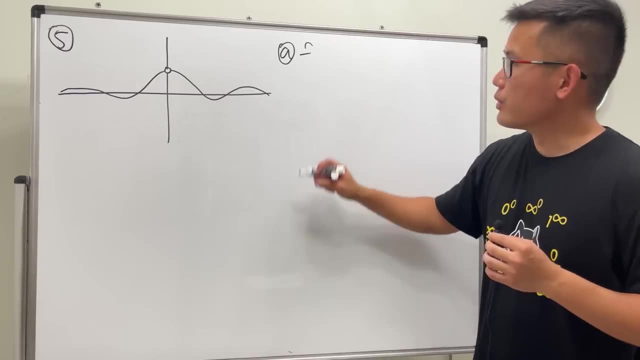 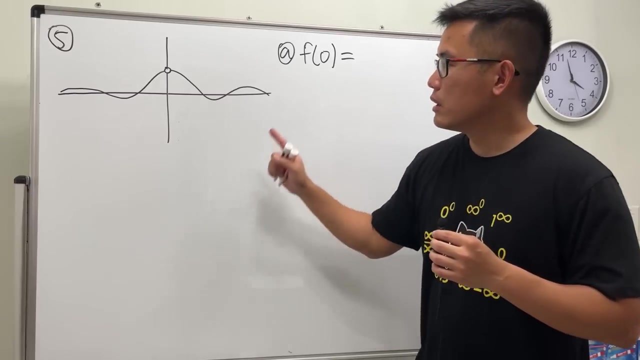 I would like to tell you guys the function. Well, no, not yet. Let me just give you guys the questions. first, Let's go over them without knowing what the function is. Firstly, what's f of zero Here? If you look at this right here, f of zero when x is zero. 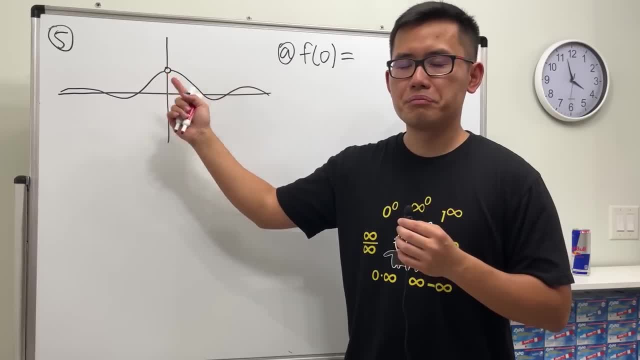 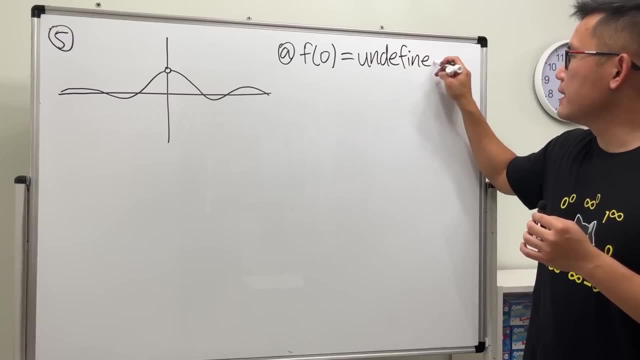 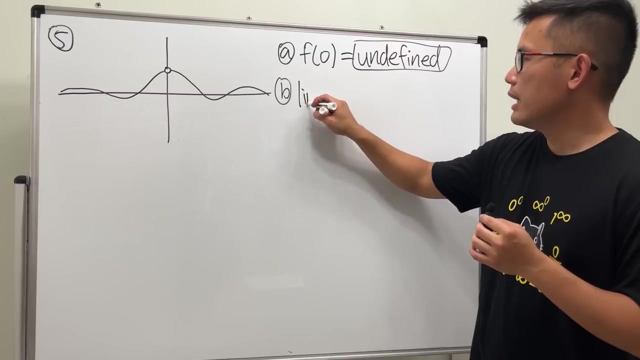 which is right here. if you look up, that's just an open circle. There's no answer for that right. So f of zero, right here, is undefined. So that's the answer for that. Okay, All right. And then, if you look at part b, if we do the limit as x approaching zero of the function, 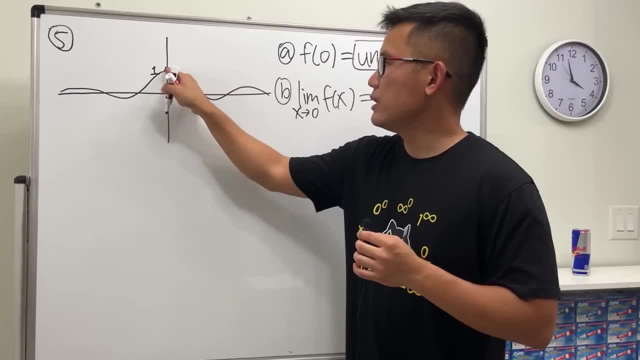 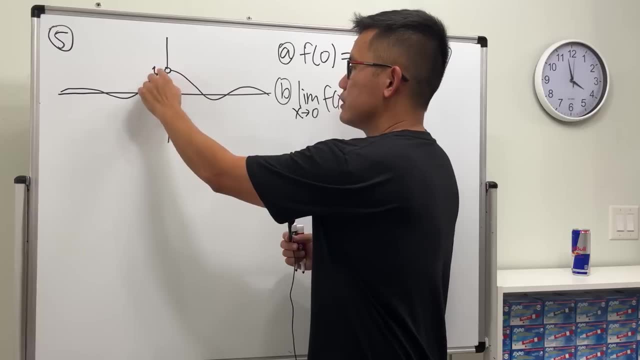 this right here. if you look at the y-foil here, it's actually one. So if you approach from the right, the y-foil is one. If we approach from the left, the y-foil is also approaching one. 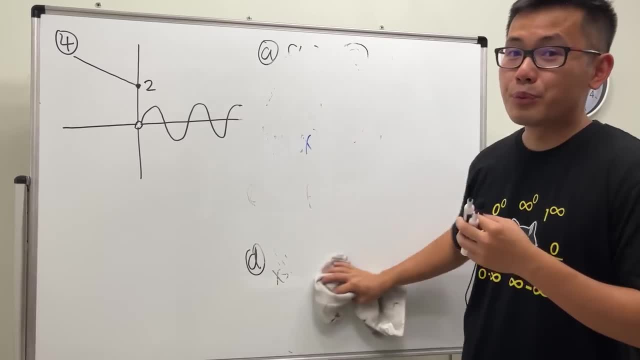 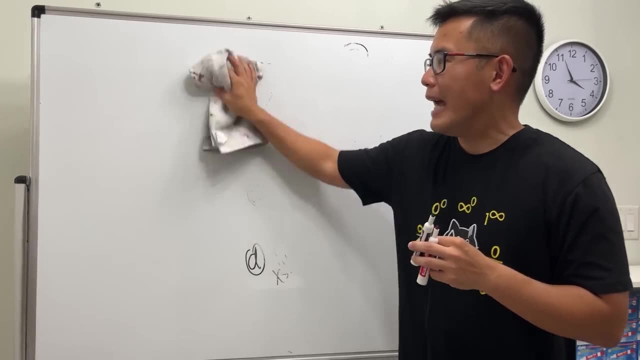 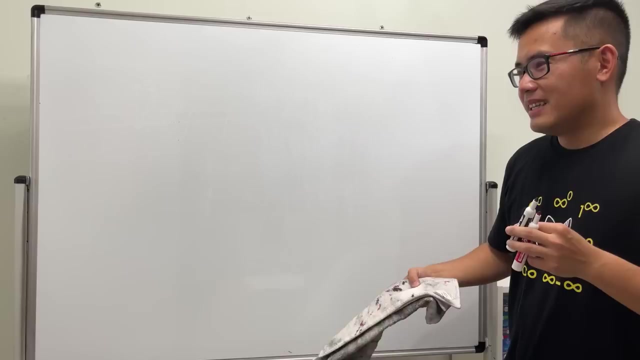 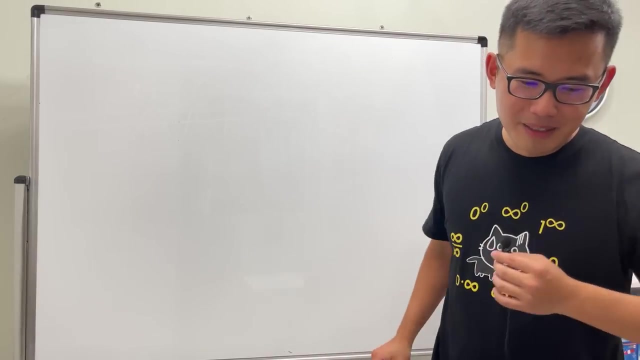 uh, it's okay, because in fact, this is my new microphone, because the previous microphone, yeah, if i don't know what happened, but i it just got bad. and uh, i i'm pretty sure it's because i dropped a lot, not well, i dropped a few times. yeah, let me just use that. i don't know how many is the last, but 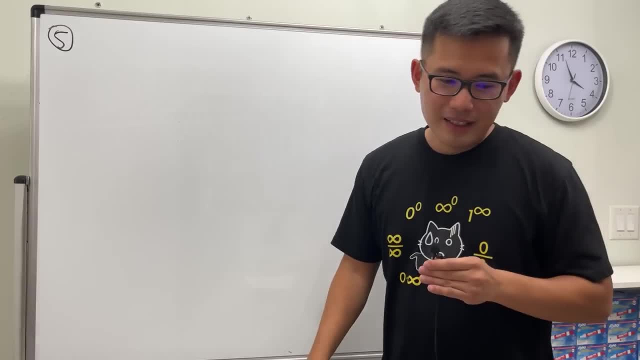 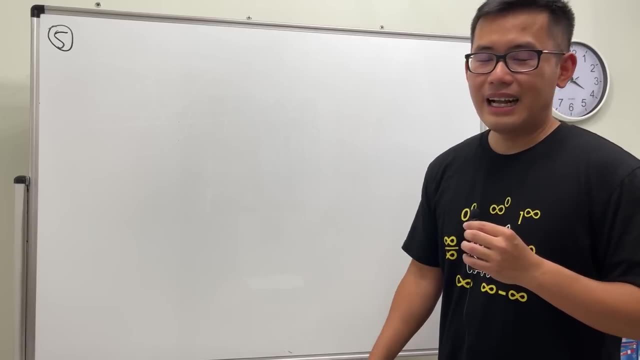 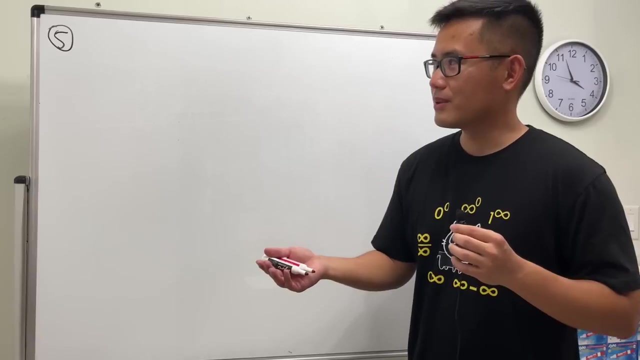 anyway, number five, number five. if, because i dropped it earlier and then the stone went back and then i broke it, that will suck, because i i cannot hear how the sound is recorded right now. this is question number five. only 96 questions to to go. anyway, all right, number five. this is the famous. 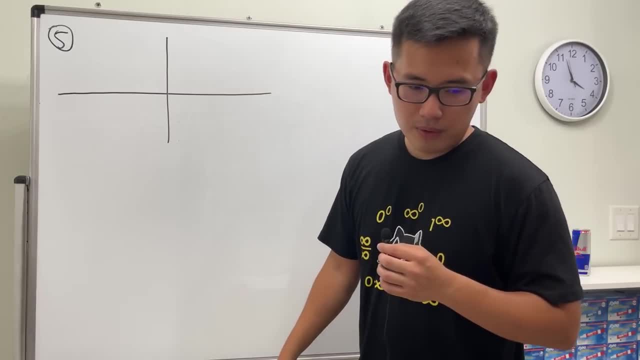 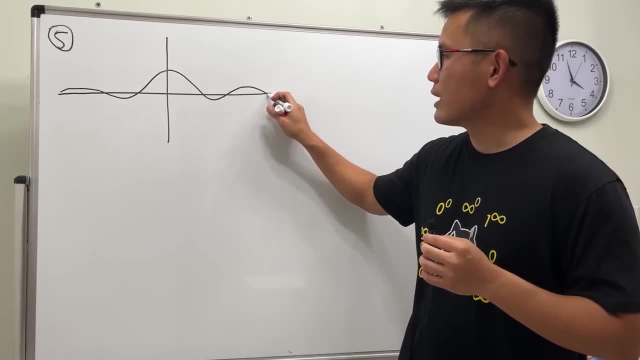 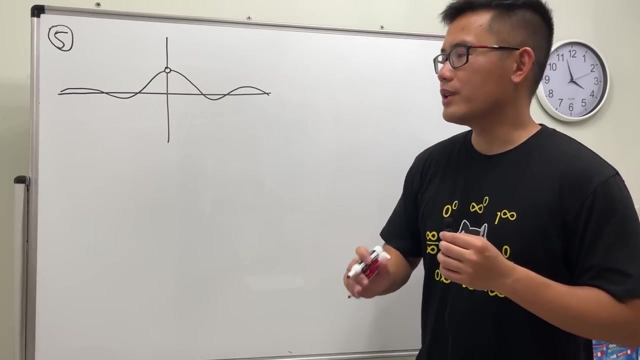 question right. so the curve looks like this, somewhat like that right, and in fact here we have an open circle. i would like to tell you guys the function, what? no, not yet. let me just give you guys the questions. first, let's go over them without knowing what the function is. 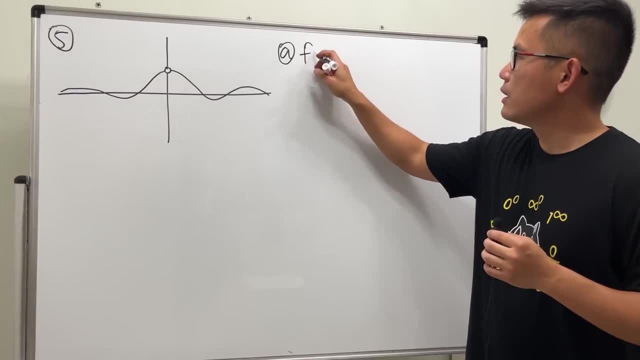 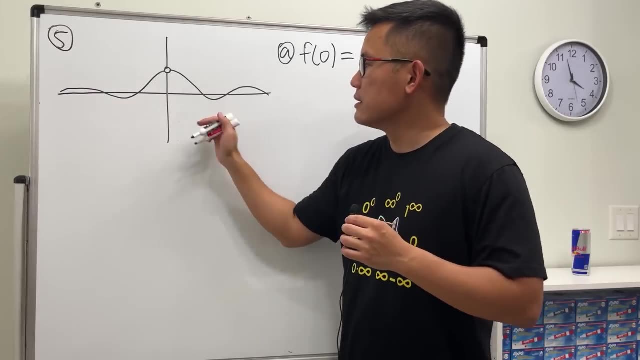 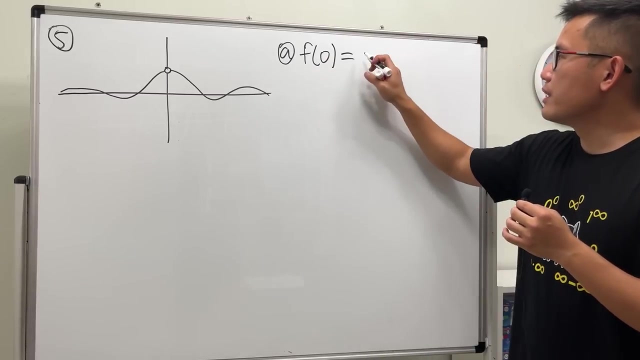 firstly, what's f of zero here? if you look at this right here, f of zero when x is zero, which is right here, if you look up, that's just an open circle. there's no answer for that right. so f of zero, right here is. and the 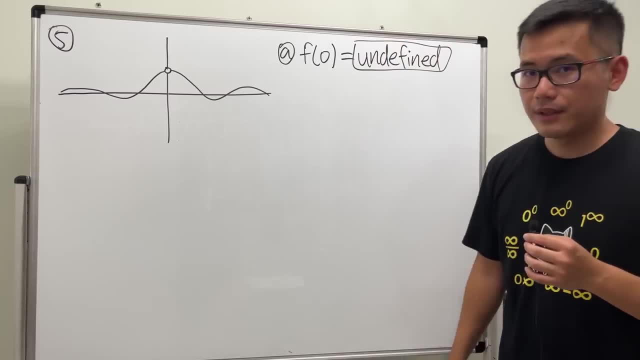 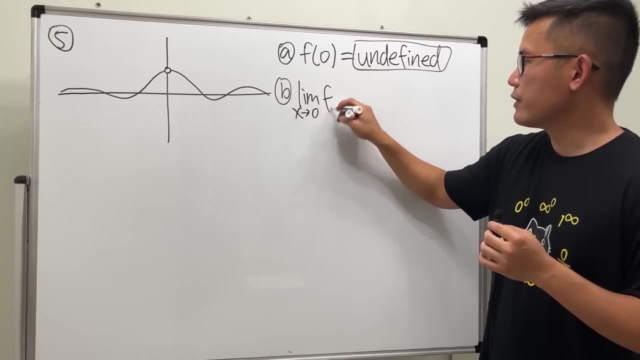 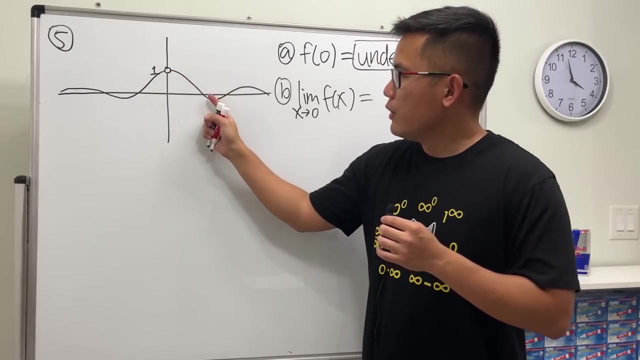 bind. so that's the answer for that, okay. and then if you take part b, if we do the limit as x, approaching zero of the function, this right here, if you look at the function of 12, the y-foil here is actually one. So if you approach from the right, the y-foil is one. 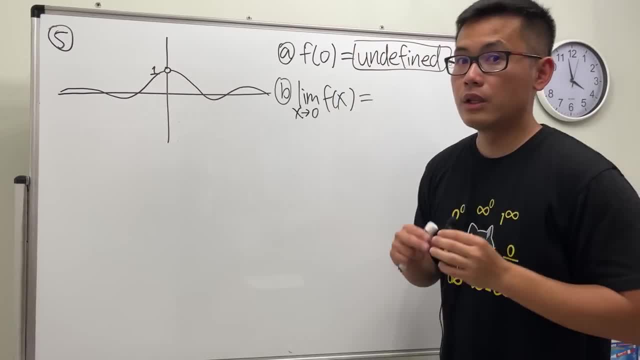 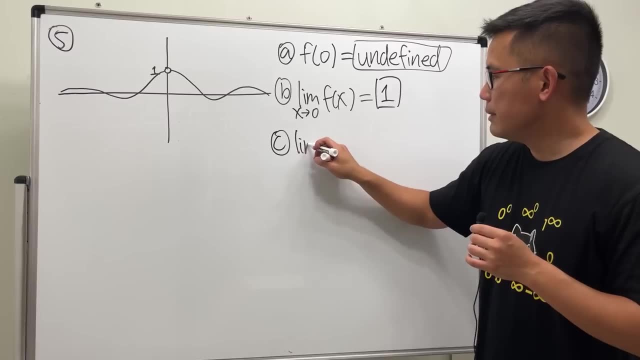 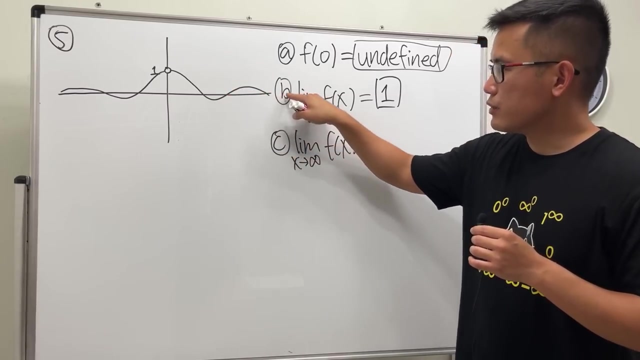 If we approach from the left, the y-foil is also approaching one. So the answer for this right here is one: All right, so that's pretty good. legit C limit. x approaching infinity. As you can see the curve, it's like this right. 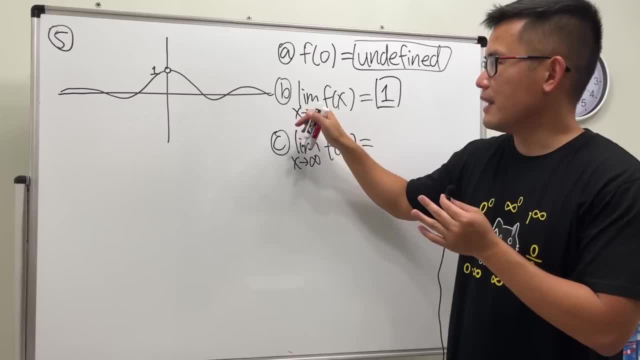 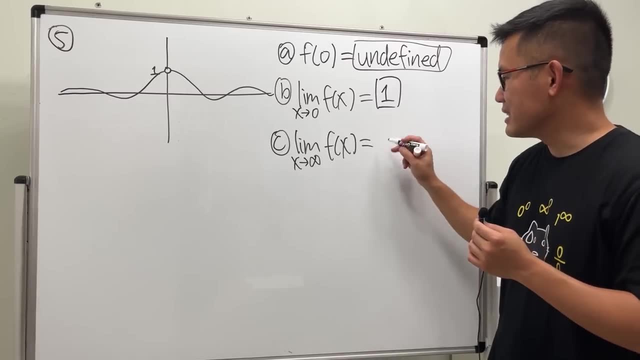 And then it's going to get like more flagged and flagged. In fact, this is not like Stein curve: The y-foil is actually approaching zero. So in this case it's zero. And again, if you look at the picture here, 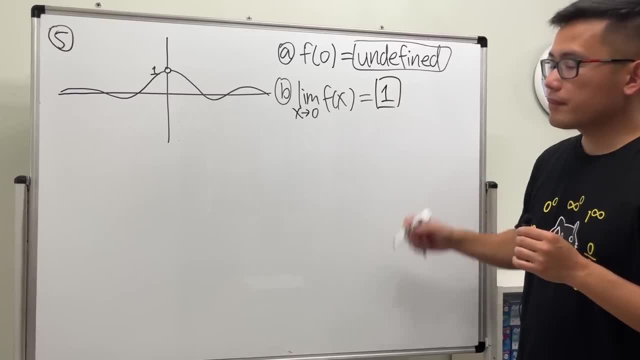 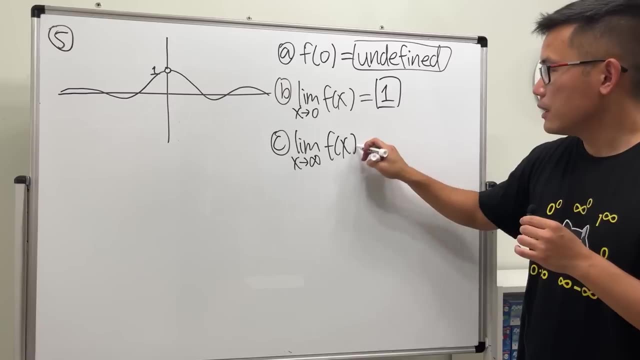 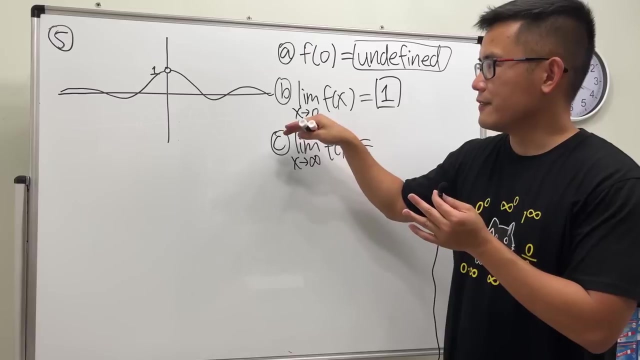 So the answer for this right here is one: All right, So that's pretty legit. That's it. C limit x approaching infinity. As you can see, the curve is like this right, And then it's going to get like more flagged and flagged. 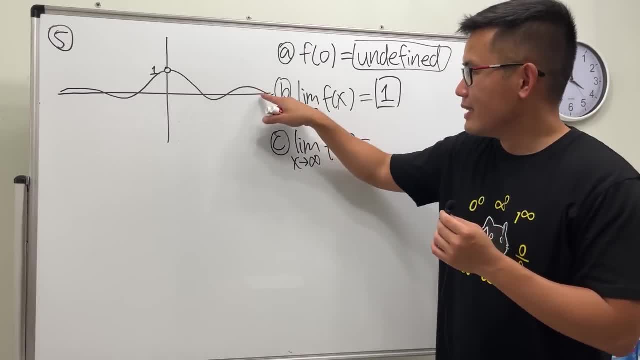 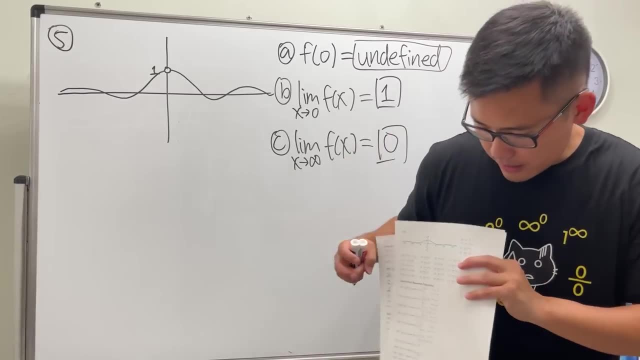 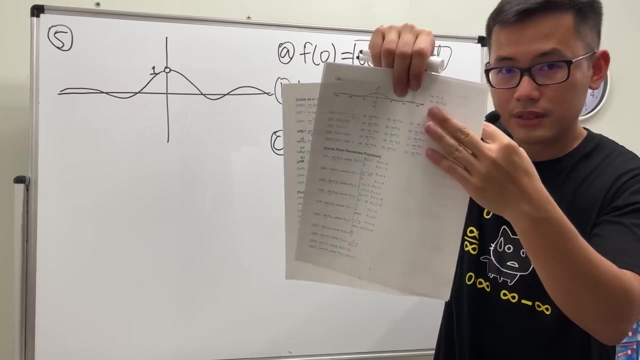 In fact this is not like Stein curve. The y-foil is actually approaching zero. So in this case it's zero And again, if you look at the picture here, it's much better to see it. right, The y-foil is just approaching zero. 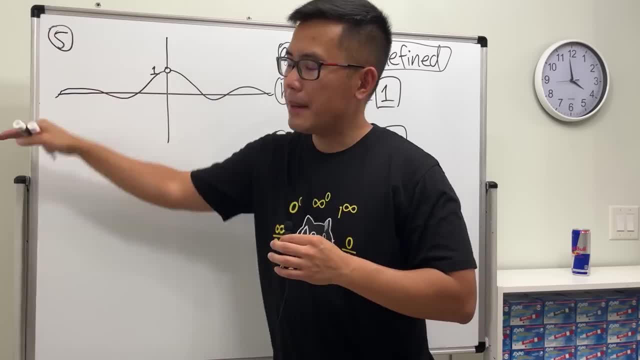 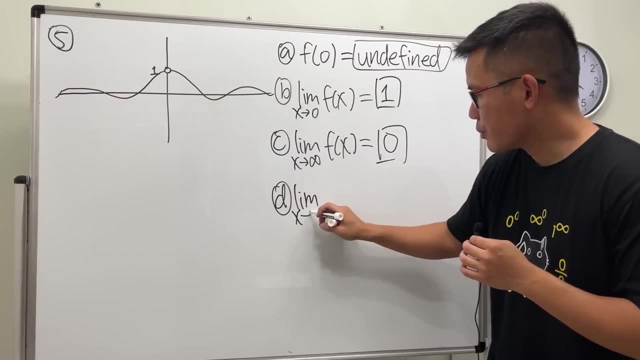 Similarly the left-hand side. It does not go up or down like that, It's not like a wave, The wave kind of dies down. So D limit x approaching negative infinity. f of x is also equal to zero. 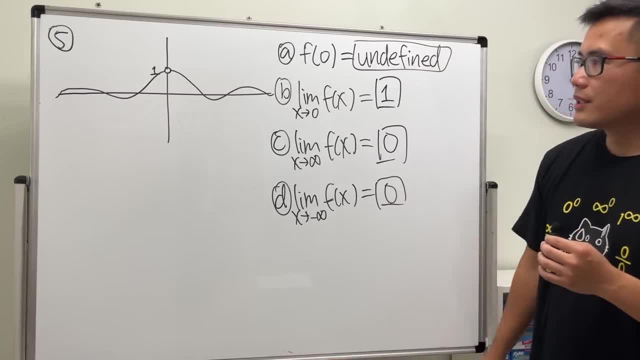 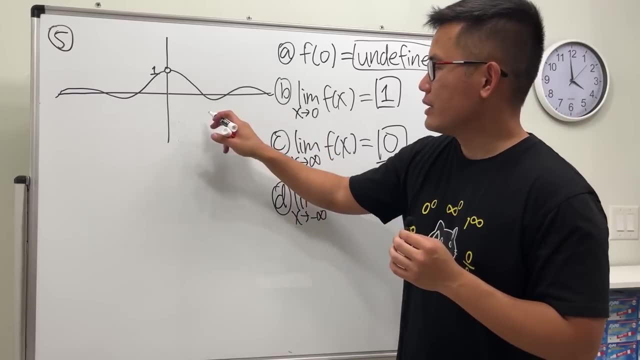 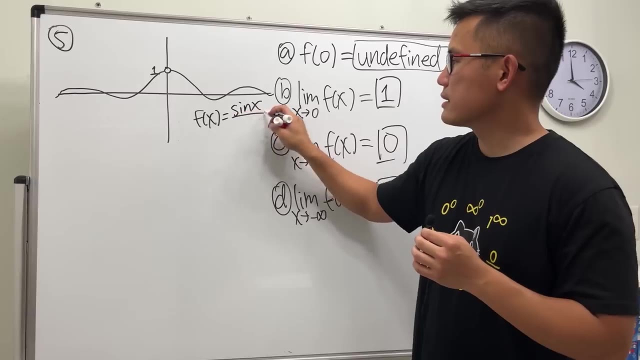 Okay, All right. So, as I said earlier, I will let you guess what this function is, because we are going to see this again later on. This function is rather famous. This is actually just f of x Equals to sine x over x. 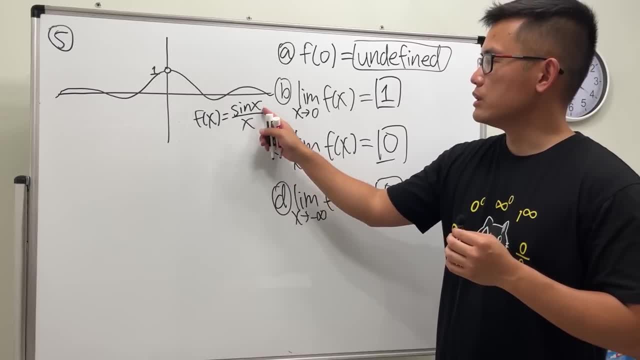 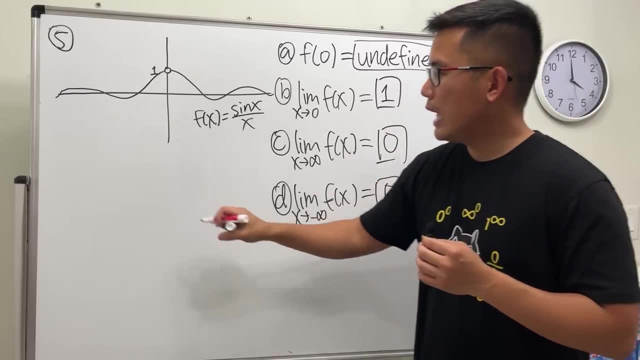 All right. So that's why you can see that when x is equal to zero, it's undefined, because we actually have a zero on the bottom, So it does not work. And then, from number two, I will let you tell you. this is what I call the limit. 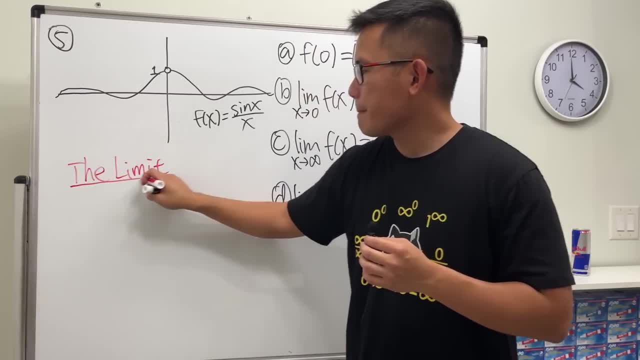 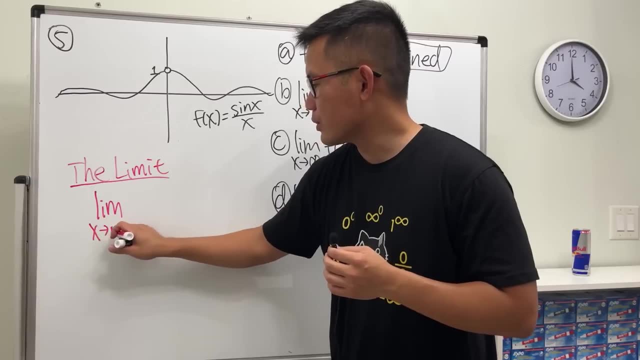 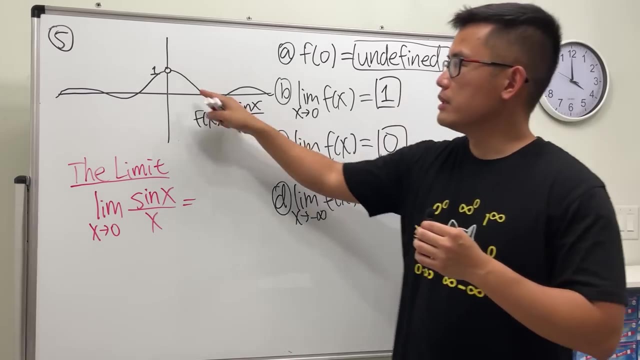 Because this is perhaps the most debatable or controversial limit, or whatnot, When we have the limit as x approaching zero. So of this function sine x over x per number two, You can see that right. Per part b, you can see that the y-value is approaching one. 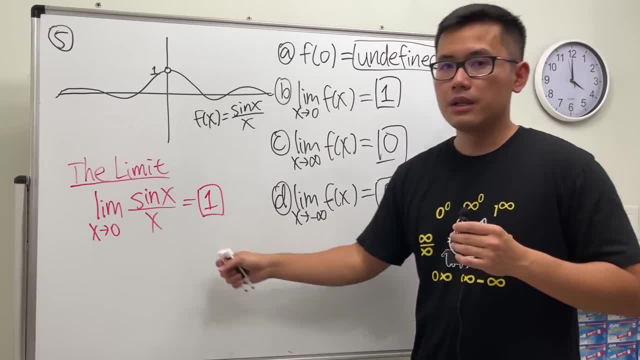 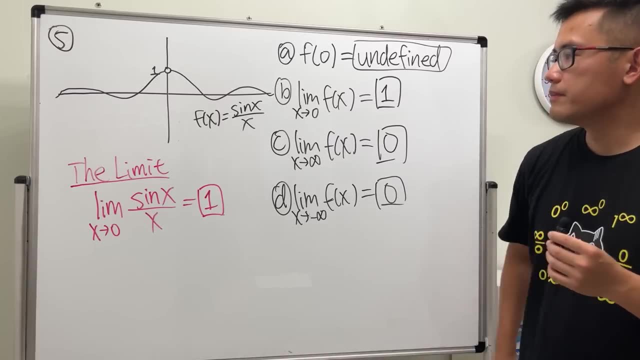 So, yeah, The answer for this right here is one: Keep this in mind. This is one of the secret weapon, And later I will just change the x to theta And you will see how we will utilize that. All right. 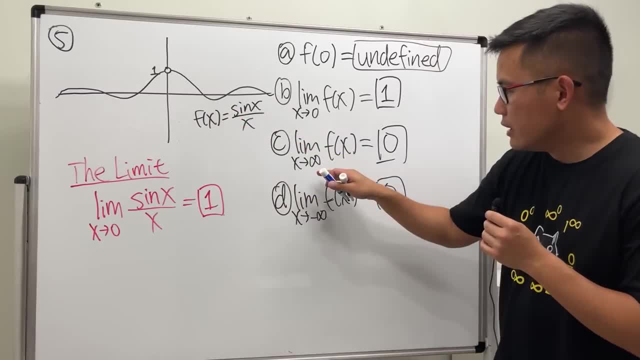 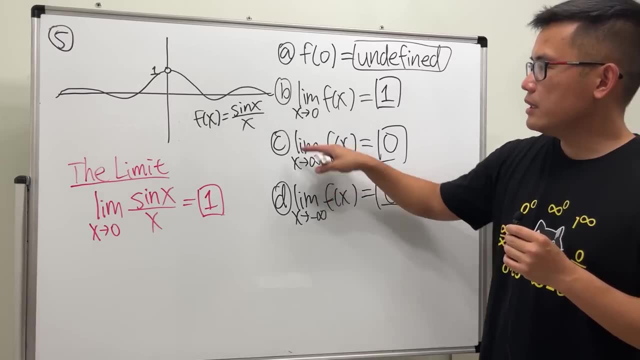 So this right here. I also want to tell you guys that the limit as x approaching zero, as x approaching infinity, is zero, likewise as x approaching negative infinity is zero. one quick way to see is you can put infinity to the top. 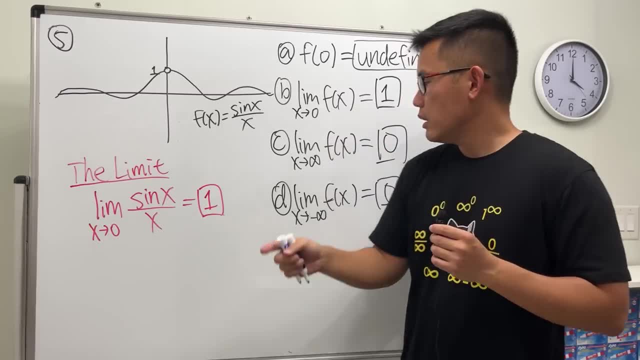 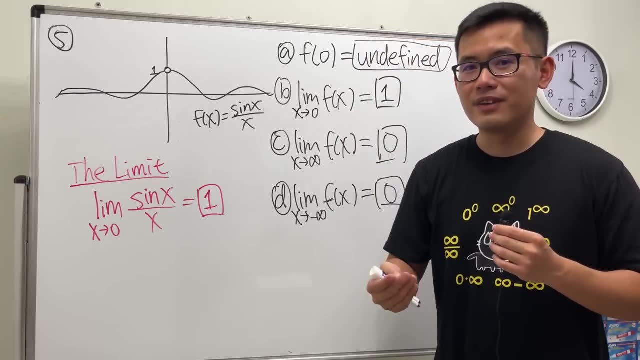 Well, sine is in between of negative one and one. But if you have infinity on the bottom, guess what It's like: one divided by infinity, which is zero, Well, negative. one divided by infinity, which is zero, Yeah, So either way, 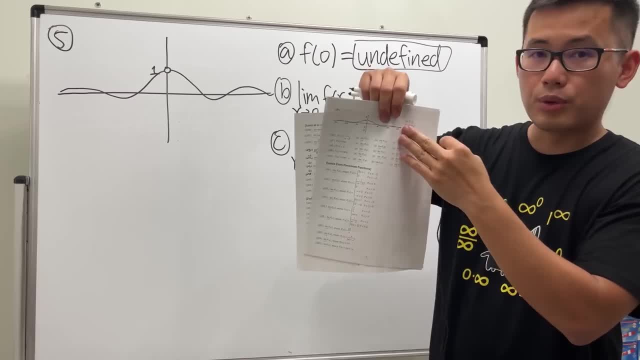 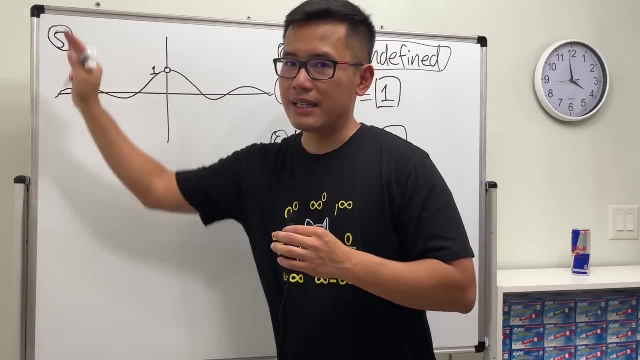 it's much better to see it right. The y-foil is just approaching zero. Similarly the left-hand side. it does not go up like down like that. It's not like a wave. The wave kind of died down. So D limit x. 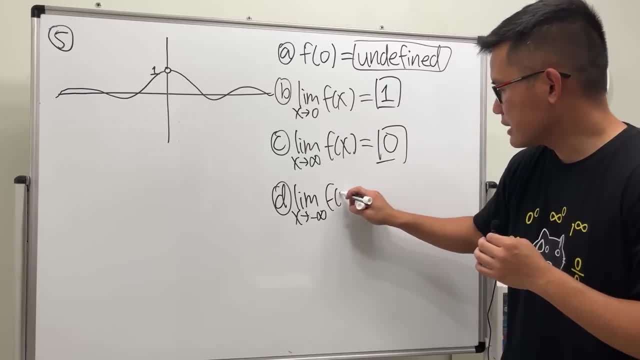 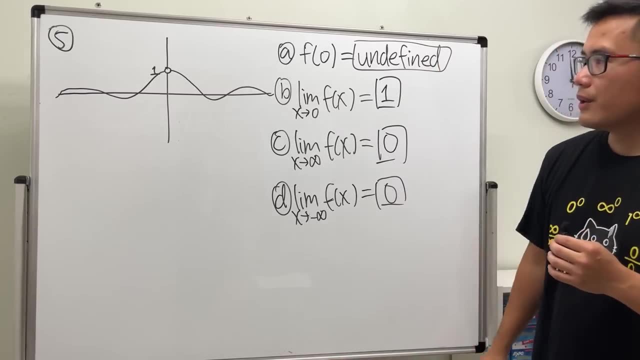 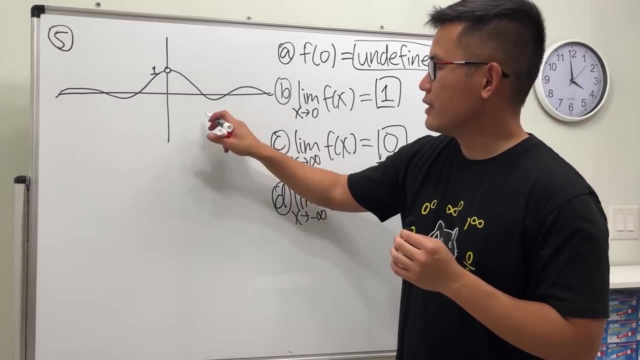 approaching negative infinity. f of x is also equal to zero. okay, All right. so, as I said earlier, I will let you guess what this function is, because we are going to see this again later on. This function is rather famous. This is actually just: f of x equals to sine x over x. 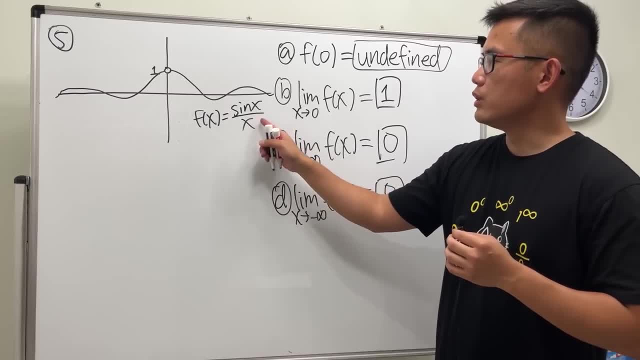 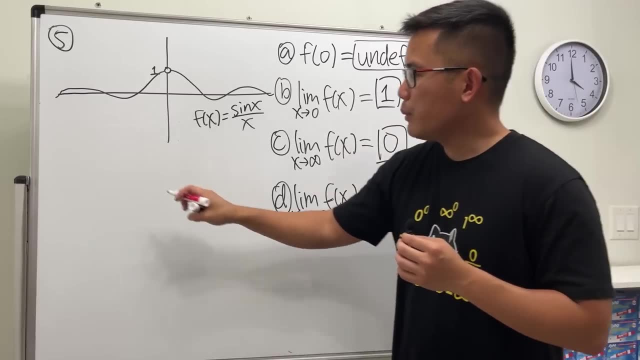 All right. so that's why you can see that when x is equal to zero, it's undefined, because we actually have a zero on the bottom, So it does not work. And then, from number two, I will let you tell you. this is why I call the limit. 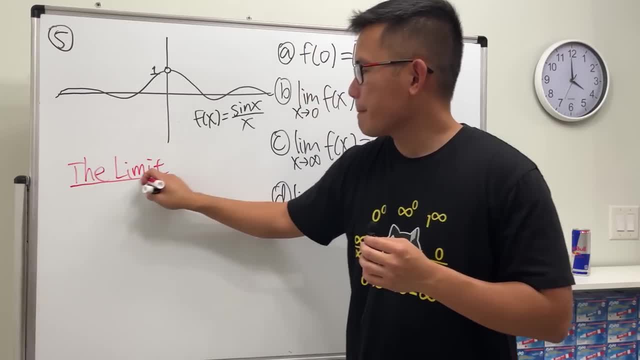 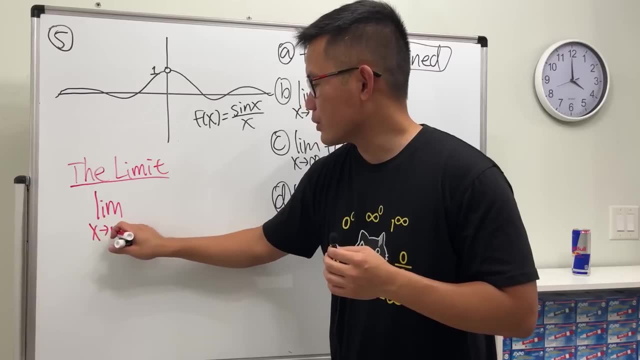 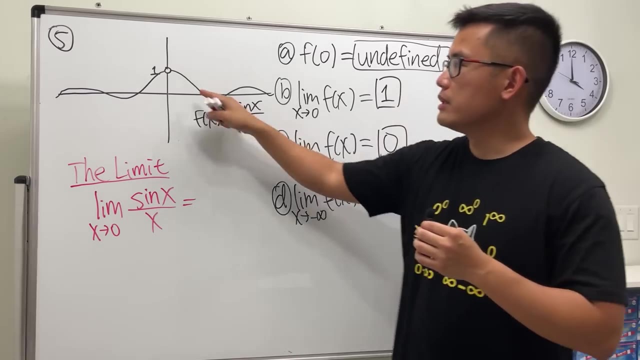 because this is perhaps the most debatable or controversial limit or whatnot, When we have the limit as x approaching zero of this function, sine x over x per number two, you can see that right. One per part b, you can see that the y-value is approaching one. 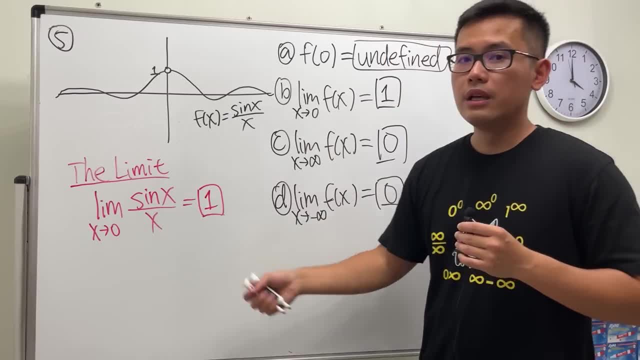 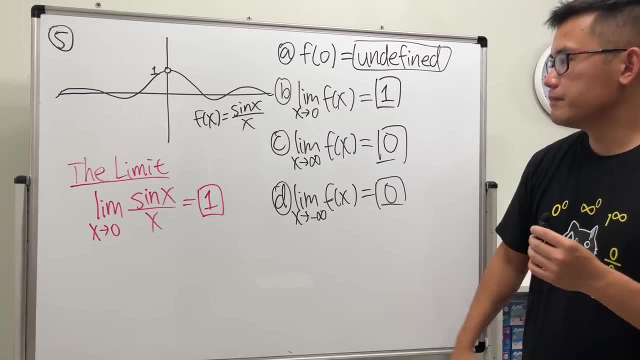 So, yeah, the answer for this right here is one: Keep this in mind: This is one of the secret weapon, And later on I will just change the x to theta and you will see how we will utilize that. All right, so this right here. 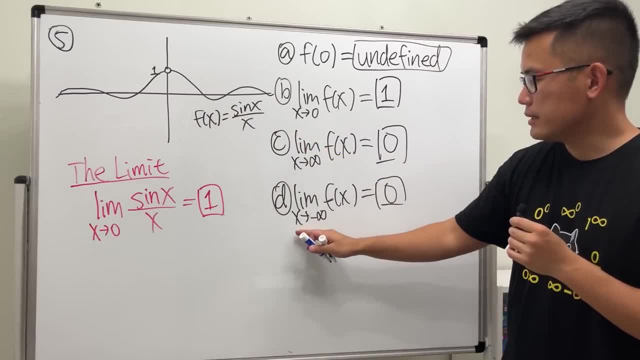 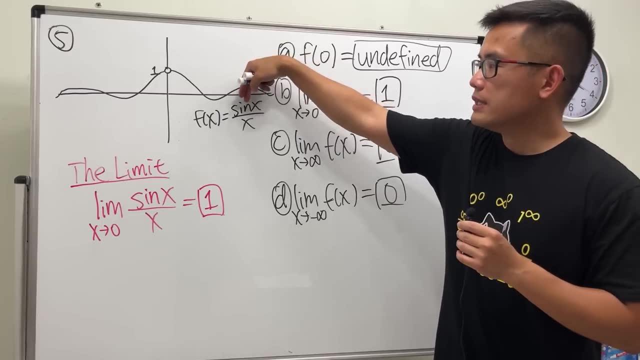 I also want to tell you guys that the limit as x approaching infinity is zero. likewise, x approaching negative infinity is zero. One quick way to see is you can put infinity to the top. well, sine is in between of negative one and one. 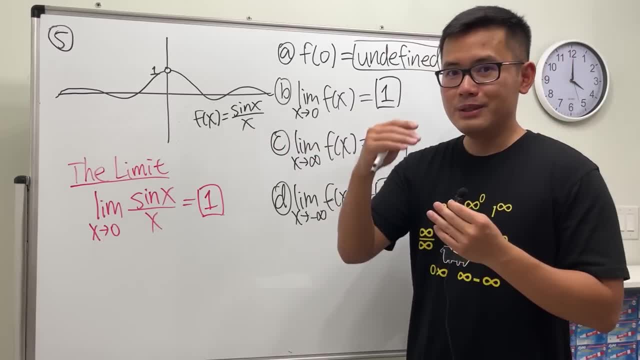 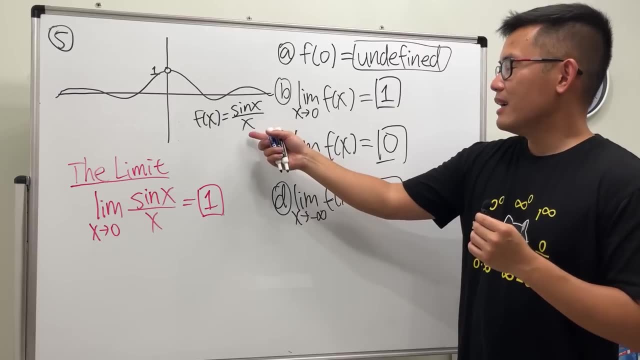 But if you have infinity on the bottom, guess what It's like: one divided by infinity, which is zero? Well, negative. one divided by infinity, which is zero, Yeah, so either way, But like, if you look at the picture, 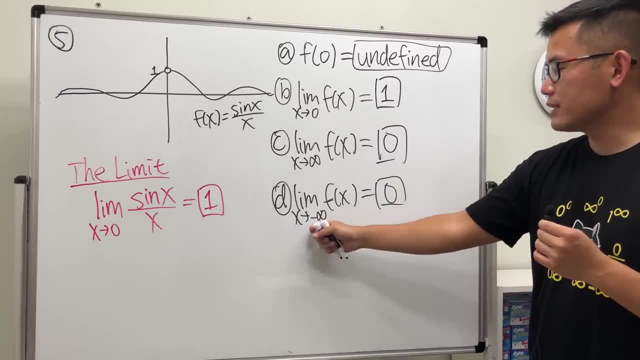 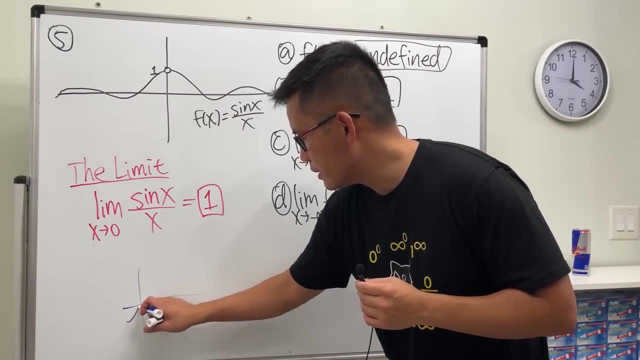 again, the wave cannot die down. that's why it's zero, And then likewise that it's also zero. However, if we look at the typical sine curve, which is like the one that we did earlier, right, So this is sine x. 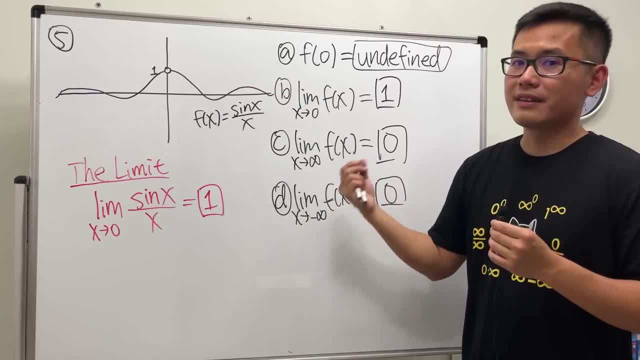 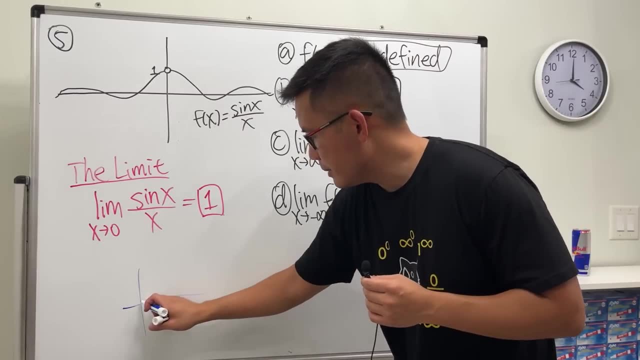 But if you look at the picture again, the wave cannot die down. That's why it's zero, And then, likewise, that is also zero. However, if we look at the typical sine curve, which is like the one that we did earlier, 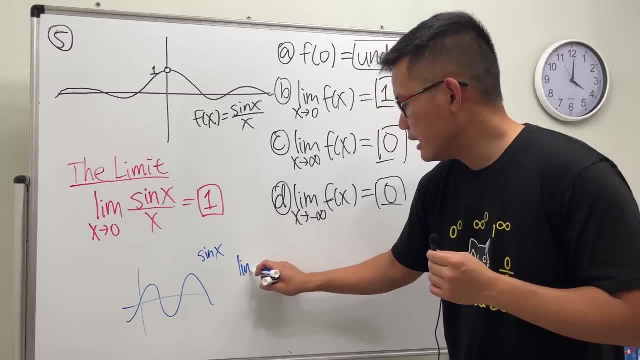 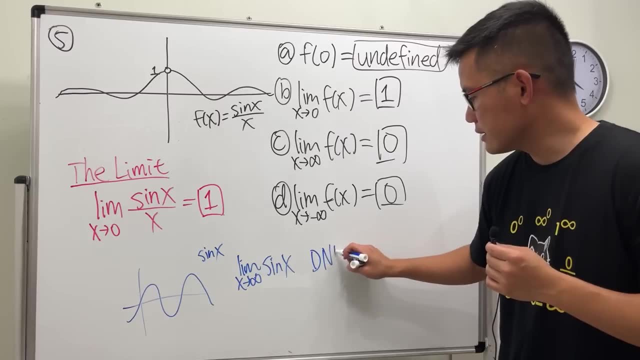 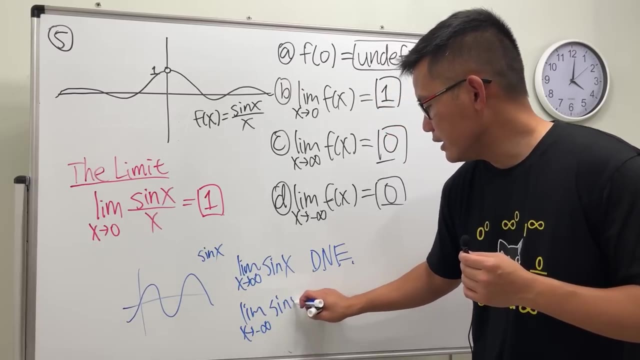 So this is sine x. Then the limit as x approaching infinity of sine x: This right here doesn't exist. It doesn't exist. Likewise the limit as x approaching negative infinity of sine x: This right here also doesn't exist. 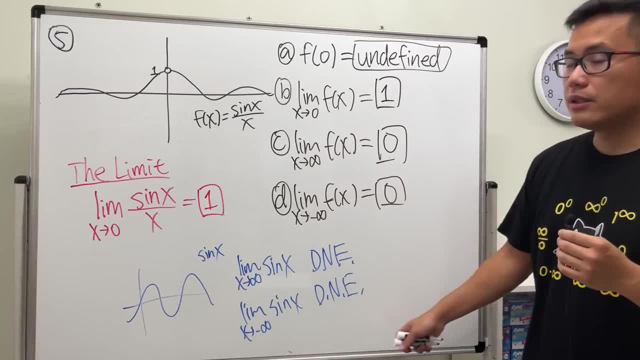 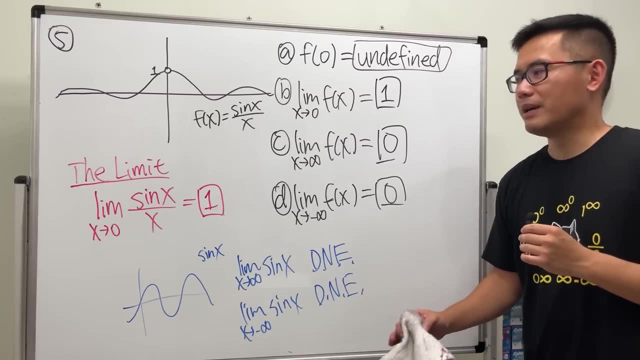 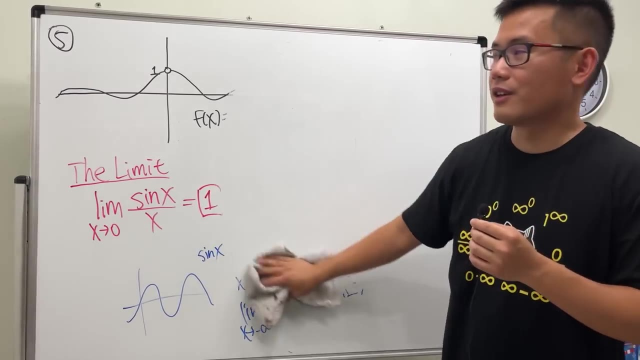 But when we divide it by the x then we end up with zero. So some of the crazier cases that you might have not seen before. because, yeah, it's the starting of calculus, So maybe you have not seen this kind of function with this kind of curves before. 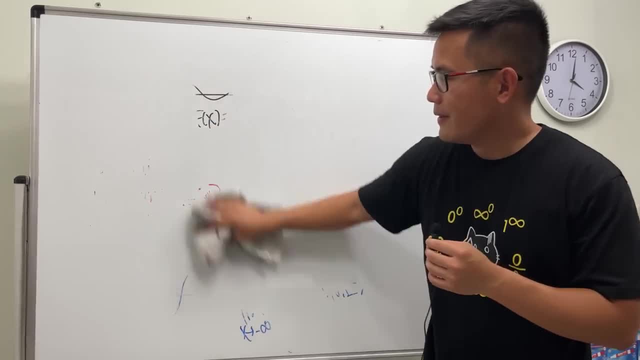 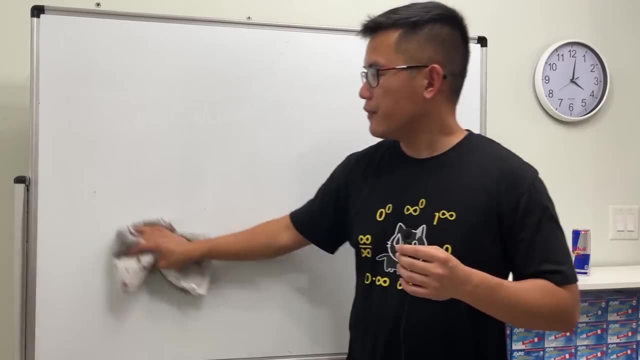 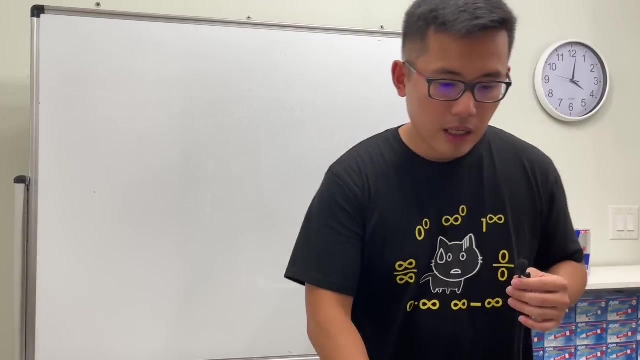 especially that one. So I want to just mention that, But we will encounter that a lot more later, Cool, So the first five questions Are the ones that I gave you guys the graph, And then you are going to figure out the limits. 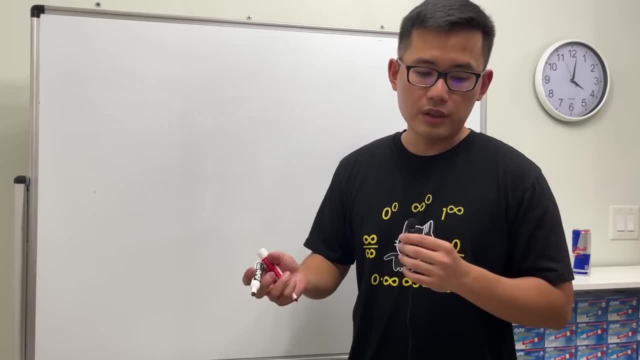 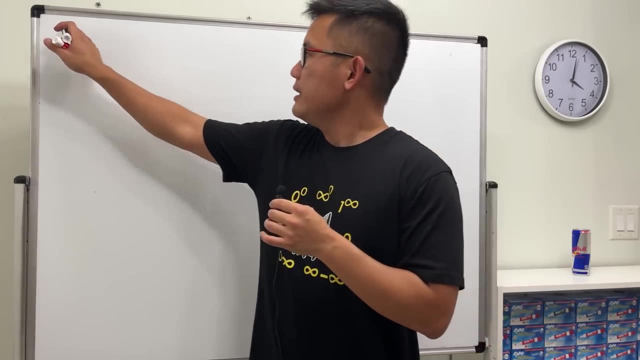 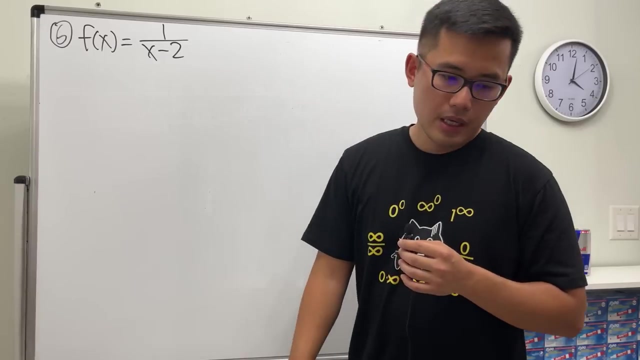 And then the next five. I will just give you guys the function, And then we are going to see how to get the limits. So, ladies and gentlemen, number six: consider we have the function, one over x minus two. You have a couple of ways to do. 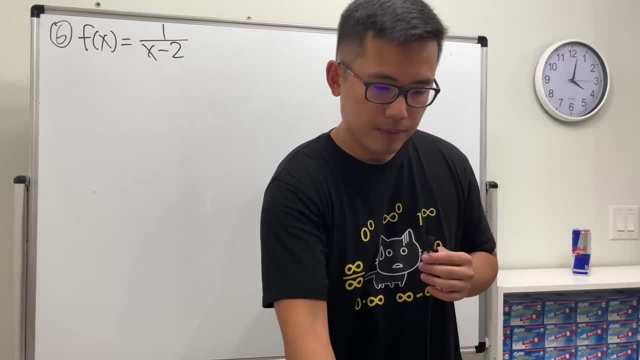 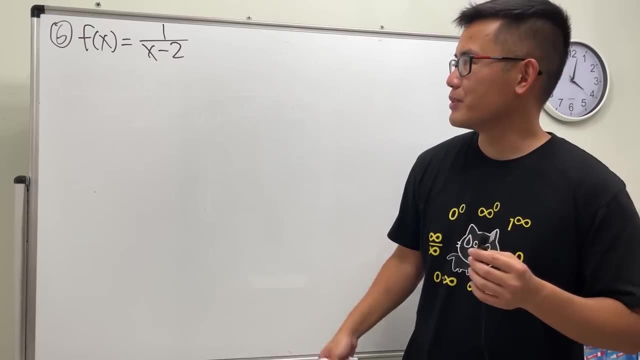 The following questions by a couple of ways. I mean like two ways. One is you come up with the graph first. Two, you don't use the graph. So kind of up to you, I will show you guys both. Let me show you how we can do it without the graph. 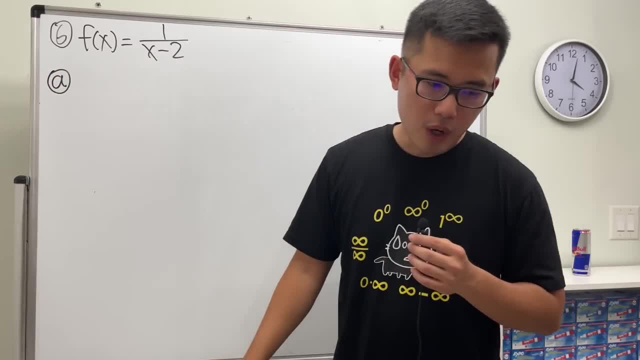 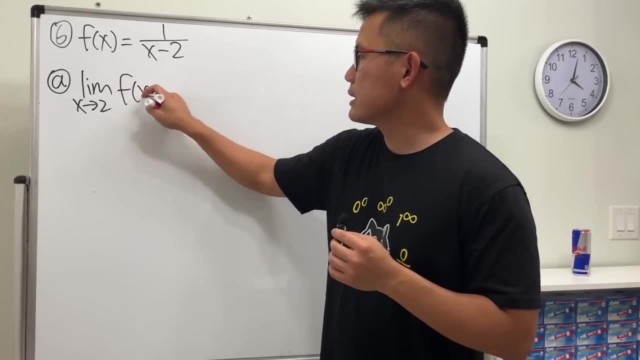 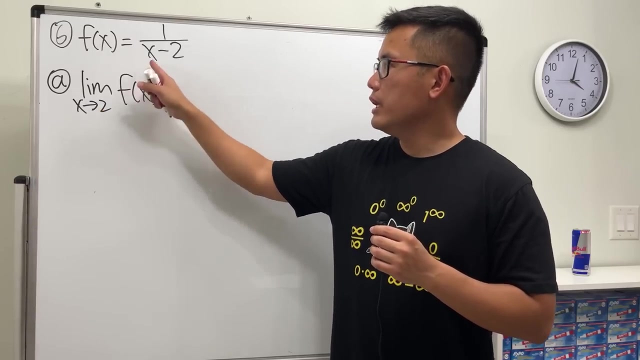 Suppose this is the function part a, We want the limit as x approaching two of the function f of x. All right, Here's the deal. If we do not use the graph, then I will just put a two into this x and see what happens. 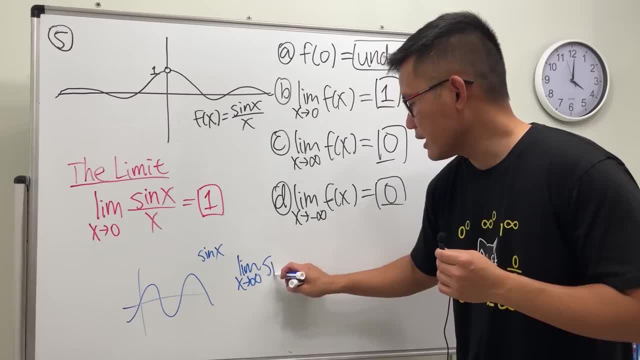 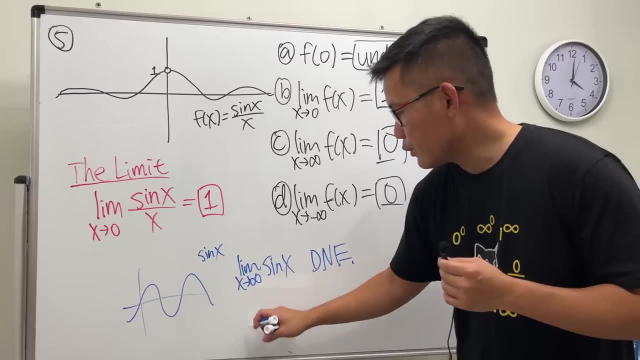 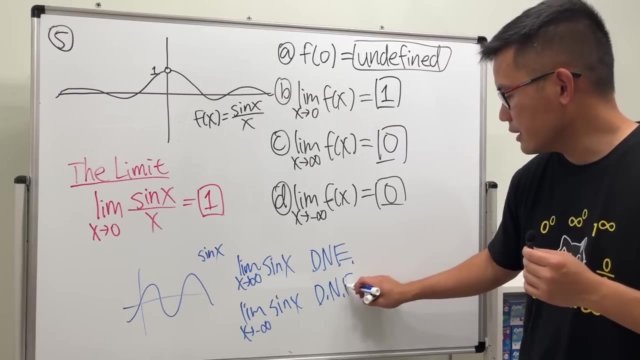 Then the limit as x approaching infinity of sine x. this right here doesn't exist. right Doesn't exist. Likewise the limit as x approaching negative infinity of sine x. this right here also doesn't exist. But when we divide it by the x, then we end up with zero. 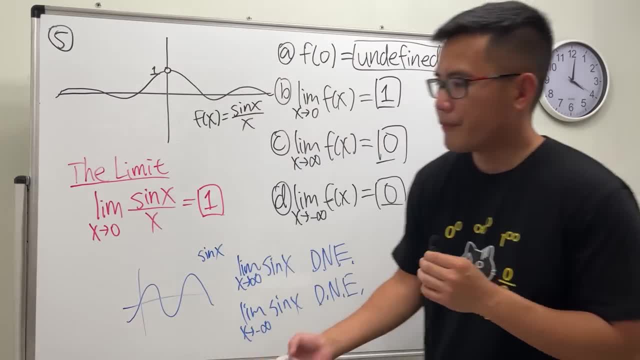 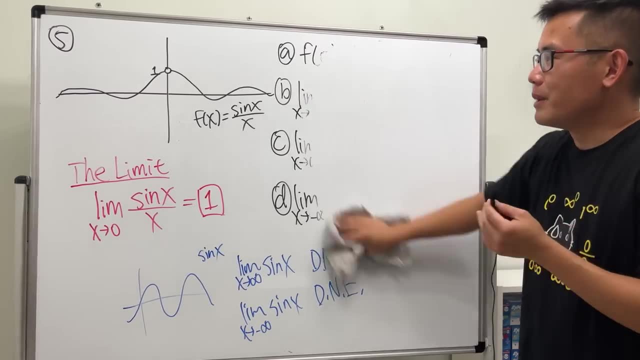 So some of the some of the crazier cases that you might have not seen before, because, yeah, it's the starting of calculus. So maybe you have not seen this kind of function with this kind of curves before, especially that one. 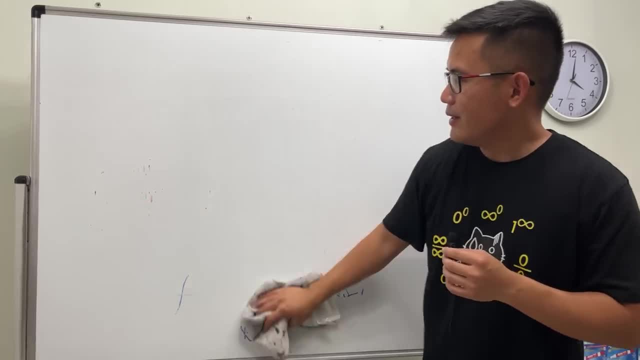 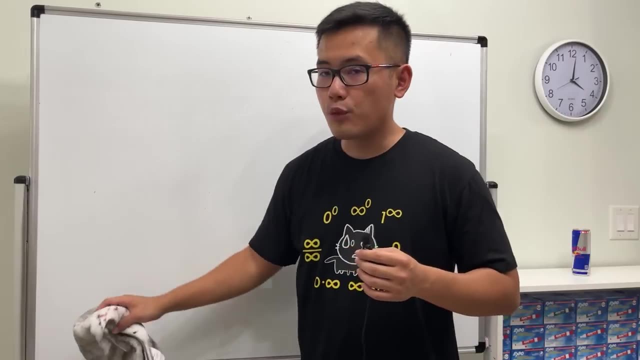 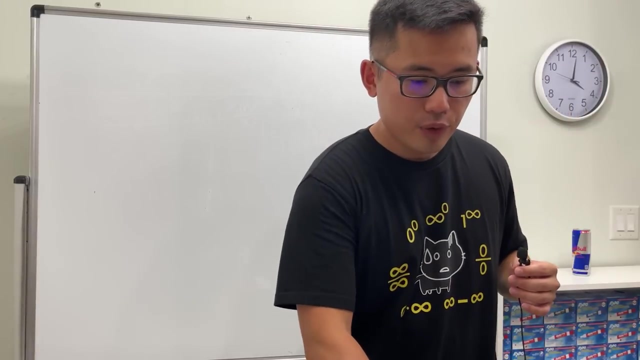 So I want to just mention that, But we will encounter that a lot more later. Cool, So the first five questions are the ones that I gave you guys the graph, And then you are going to figure out the limits, And then the next five. 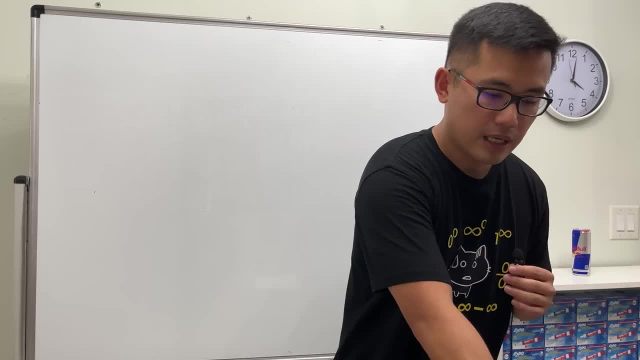 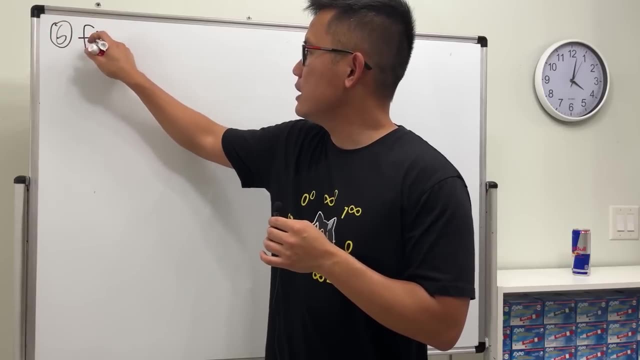 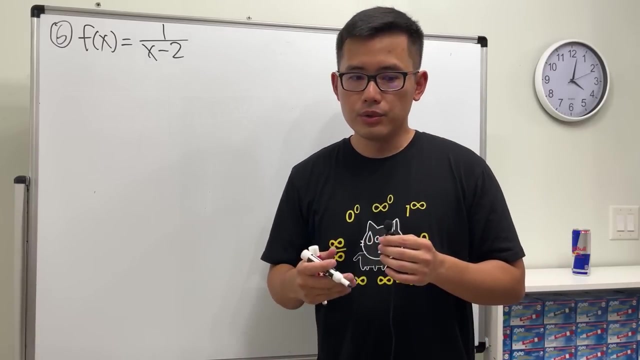 I will just give you guys the function and then we are going to see how to get the limits. So, ladies and gentlemen, number six: consider we have the function. one over x minus two. You have a couple ways to do the following questions. 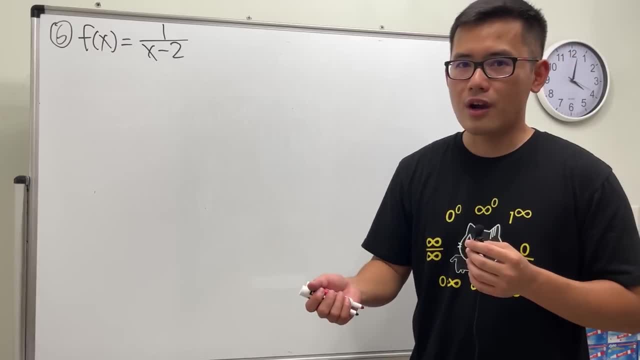 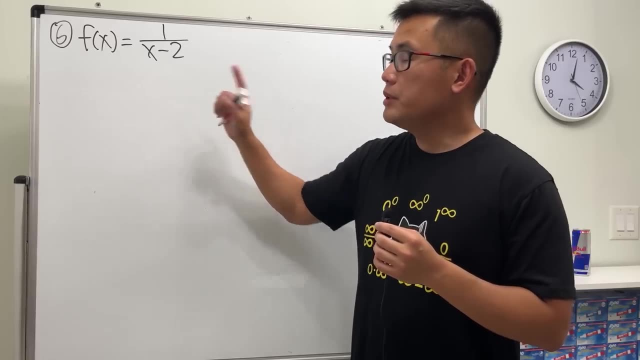 By a couple wait. I mean like two ways. One is you come up with the graph First two, you don't use the graph. So kind of up to you, I will show you guys both. Let me show you how we can do it without the graph. 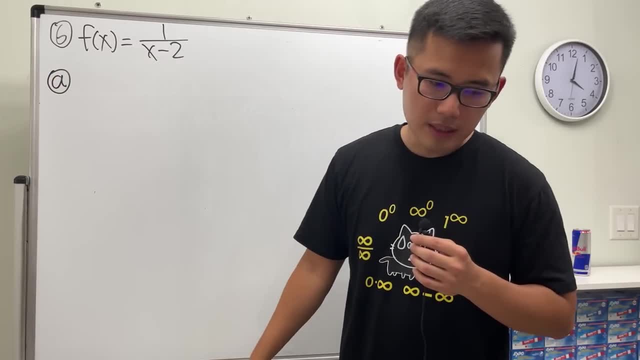 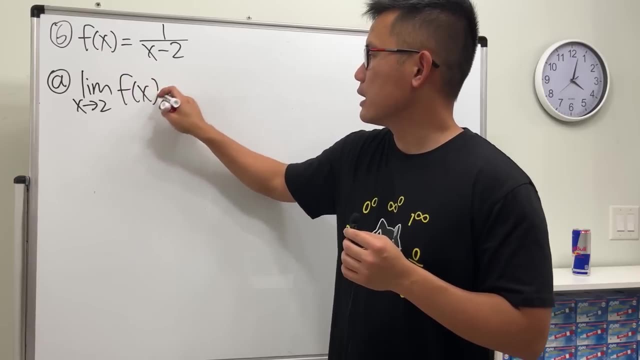 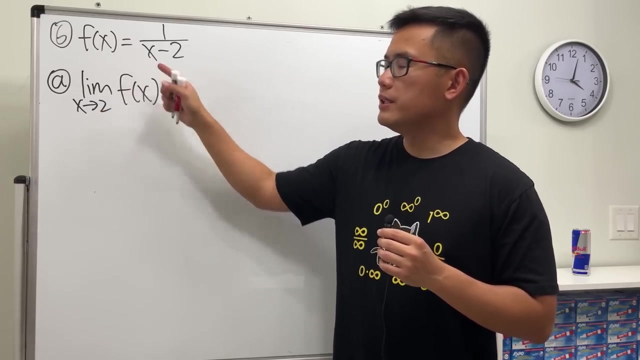 Suppose this is the function part a, we want the limit as x approaching two Of the function f of x. All right, here's the deal. If we do not use the graph, then I will just put a two into this x and see what happens. 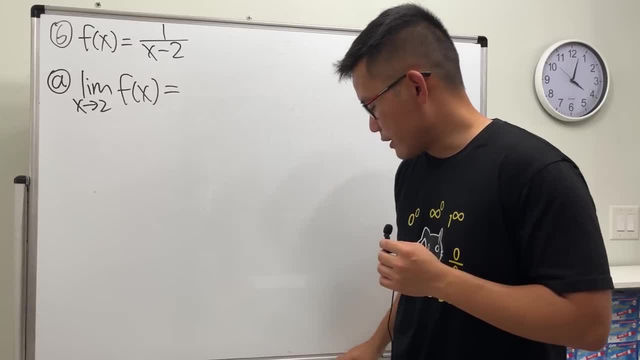 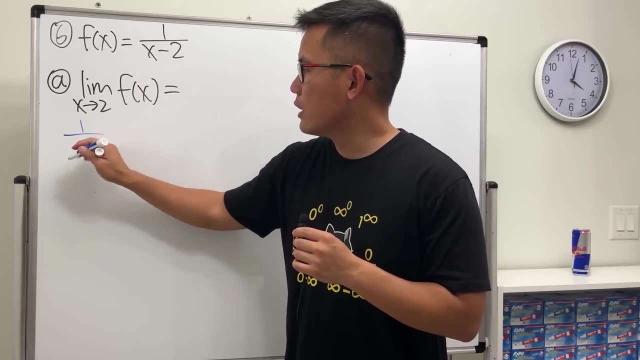 And if I do that I will get two. If I do that, I will just do some scratch work right here on the side, because this is not like a gentleman computation. Put a two into this x, we get one over two minus two. 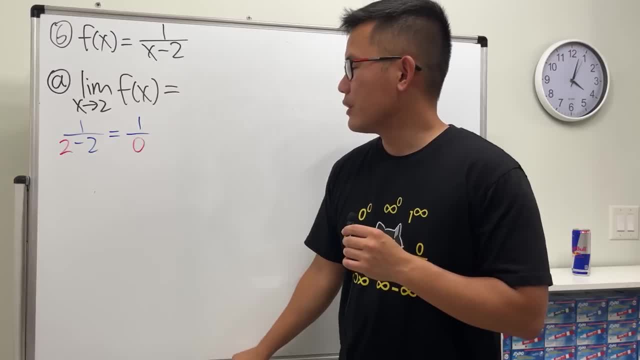 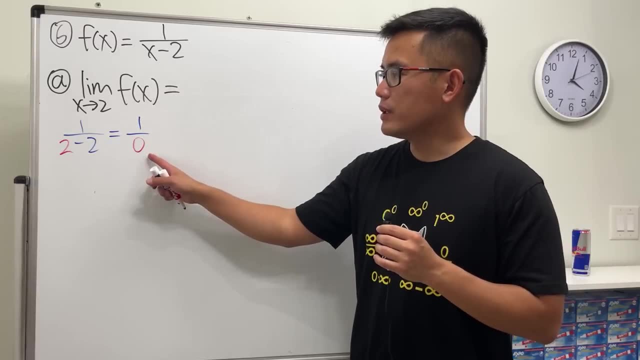 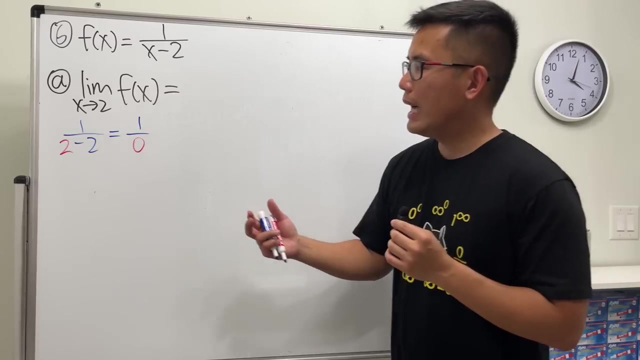 which it looks like we have one over zero, right? What does this mean? Well, let me tell you: if we have a number over zero, when we are doing limits, either we get positive infinity or negative infinity. What I mean by that is just that we will have to. 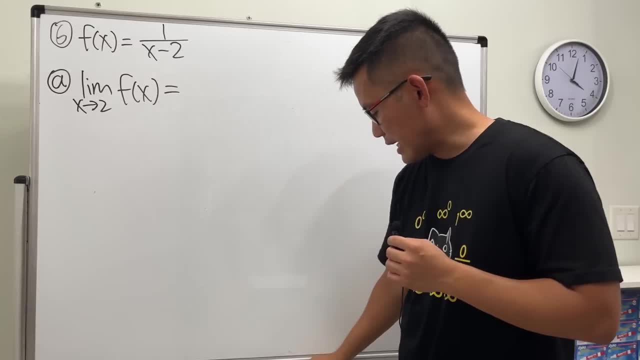 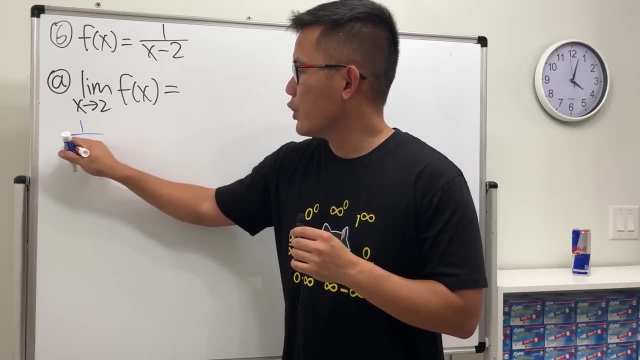 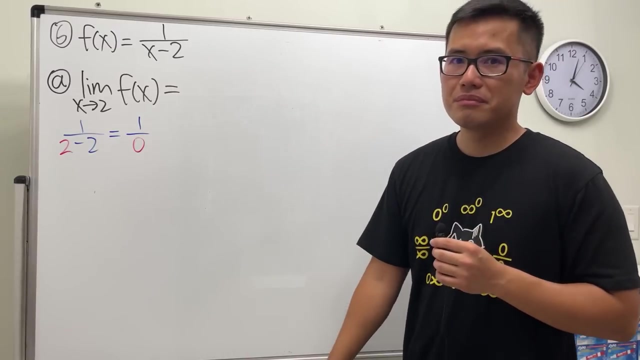 And if I do that, I'll just do some scratch work right here on the side, Because this is not like a gentleman computation. Put a two into this x, We get one over two minus two, which it looks like we have one over zero right. 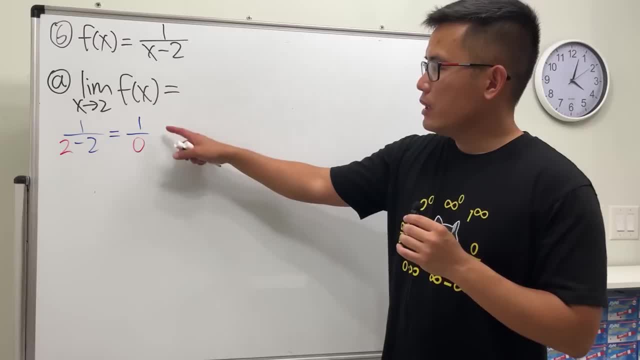 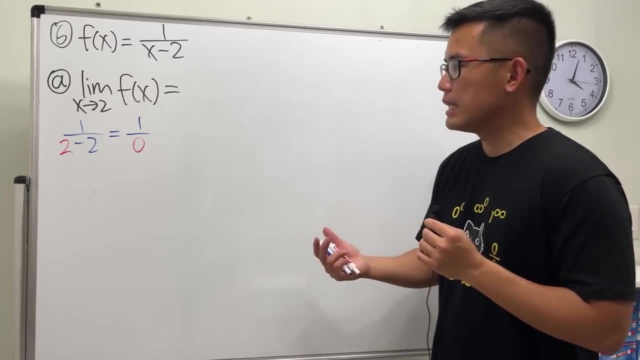 What does this mean? Well, let me tell you: If we have a number over zero and we are doing limits, either we get positive infinity or negative infinity. What I mean by that is just that we will have to worry about the sign, if it's positive or negative, when we're doing this. 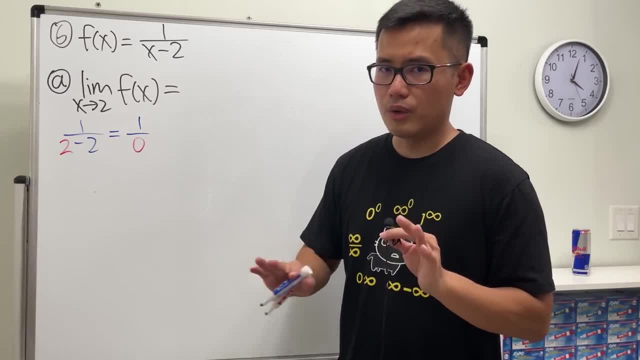 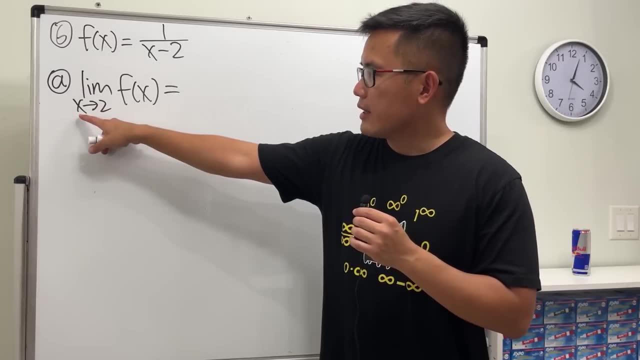 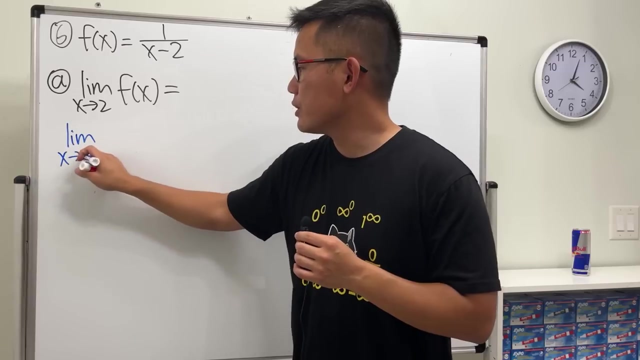 But how, though? By putting two. No, we cannot put in inside two. So that's the deal. Here's the thing Again. when x is approaching two, there's no plus or minus. We actually have to do both. Let's check the limit as x approaching two. 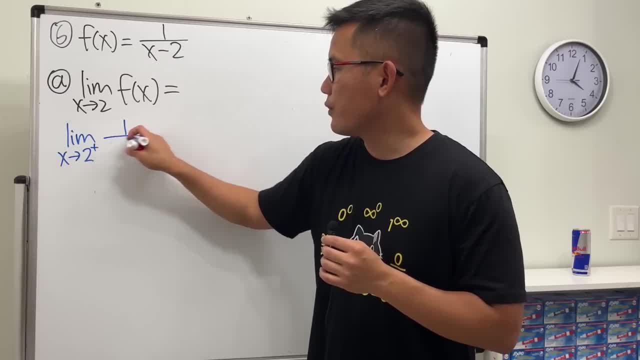 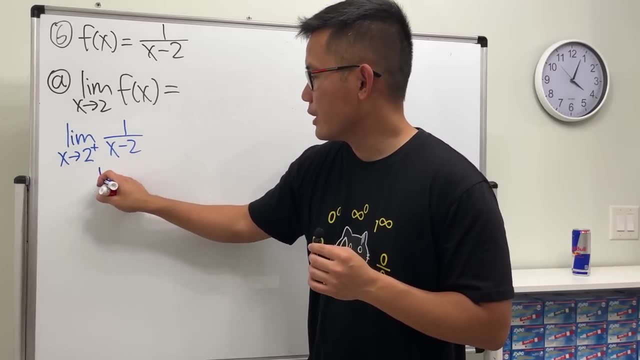 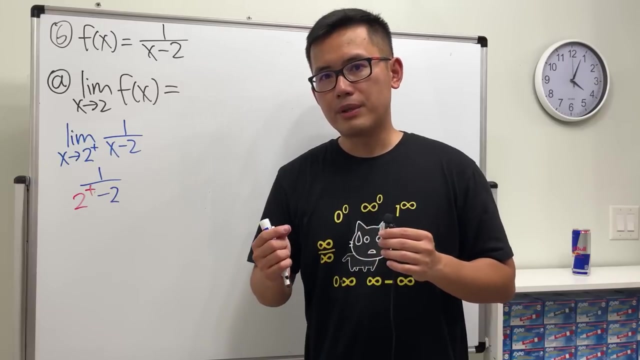 Let's do the positive version first, And then the function is one over x minus two. Yeah, So let's see, When we put two plus into here, we are going to get one over two plus minus two. Two plus is just like a number slightly bigger than two. 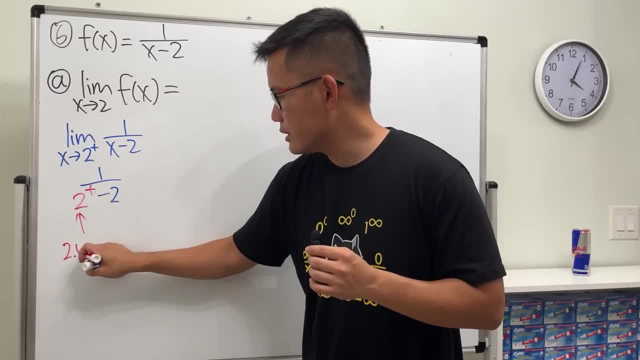 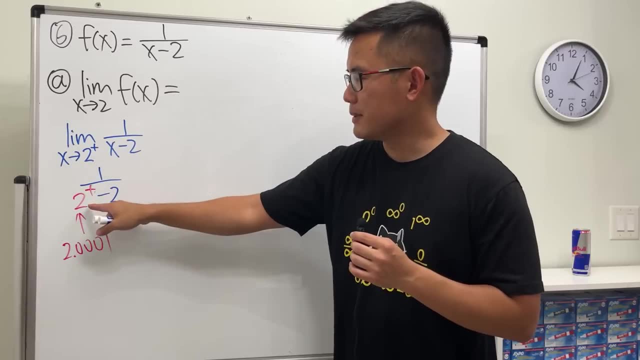 Just think about it like that And you can think about it as two point zero, zero zero one. So earlier, when we do like two minus two, not so much, This is better: Two plus minus two. This right here is approaching zero. 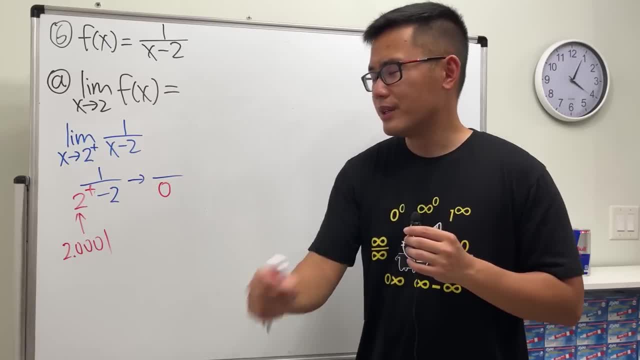 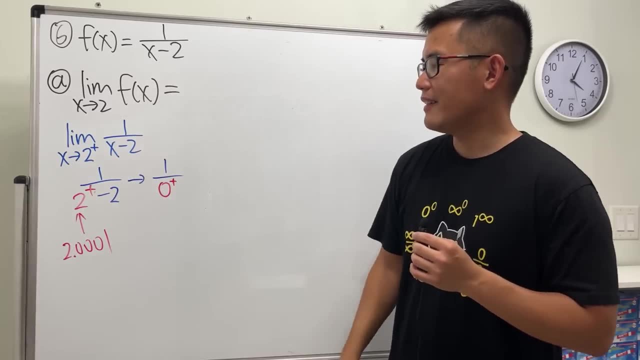 Two minus two is zero, But this right here is a little bit more than two. So this zero is actually a little bit more than zero. So this is technically zero plus OK. And then on the top we still have the one. 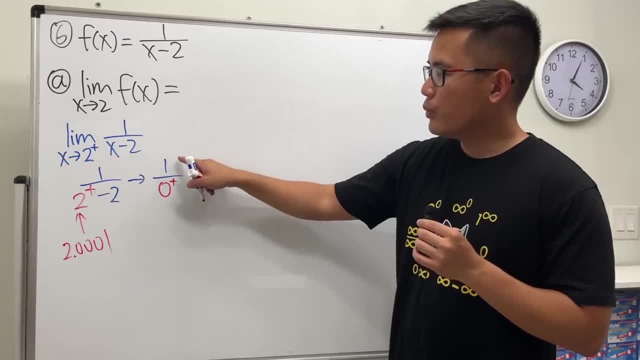 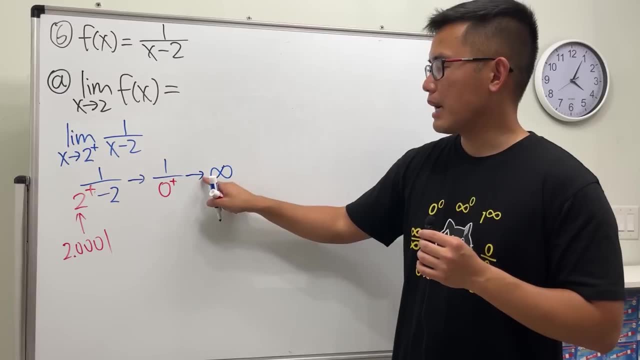 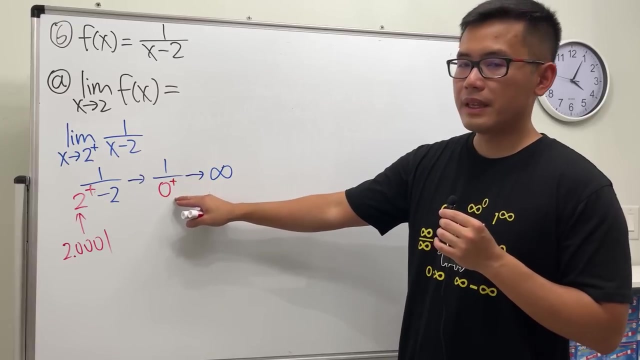 So we have one over zero plus, And when we have one over zero plus, when we're doing limits this right here- positive over positive, we get positive, And then you get infinity. Whenever we are doing this kind of computation, if we have a zero plus or zero minus on the bottom, if the top is non-zero, 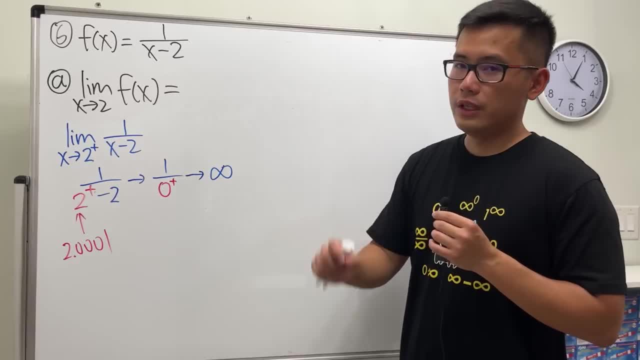 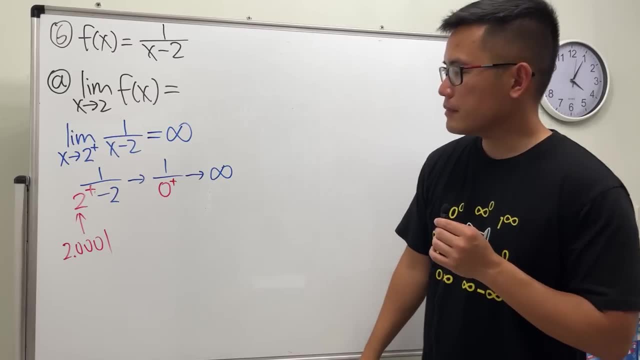 then you are going to expect to get either positive infinity or negative infinity, And again just work out the sign. So this right here gives us positive infinity, OK, And then let's see if we have the limit as x approaching, two minus and then one. 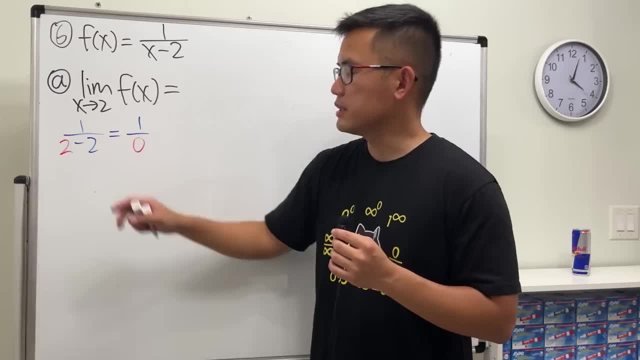 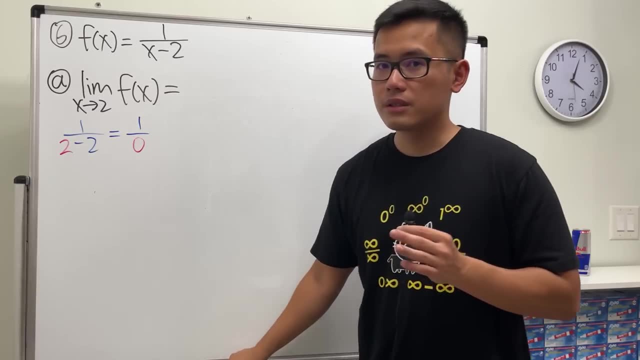 worry about the sign, if it's positive or negative, when we're doing this. But how though I put in two? No, we cannot put in inside two. So that's the deal. Here's the thing Again, when x is approaching two. 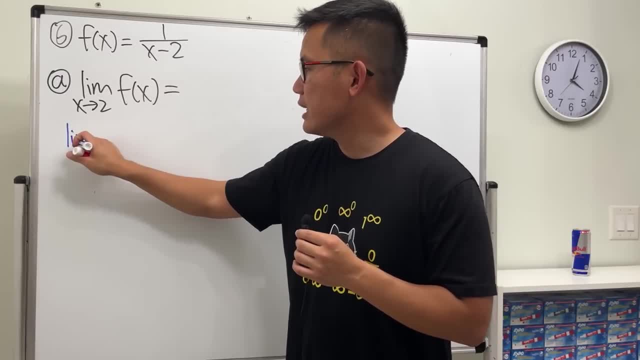 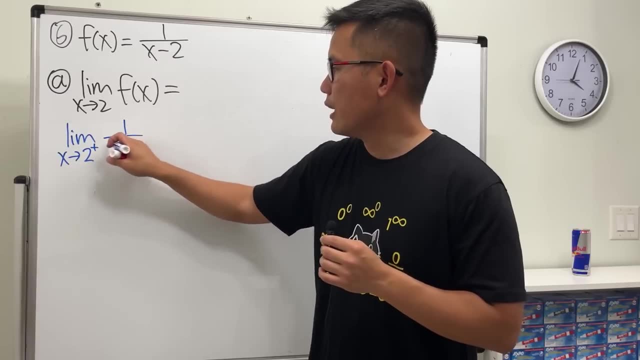 there's no plus or minus. we actually have to do both. Let's check the limit as x approaching two. Let's do the positive version first, And then the function is one over x minus two. yeah, So let's see When we put two plus into here. 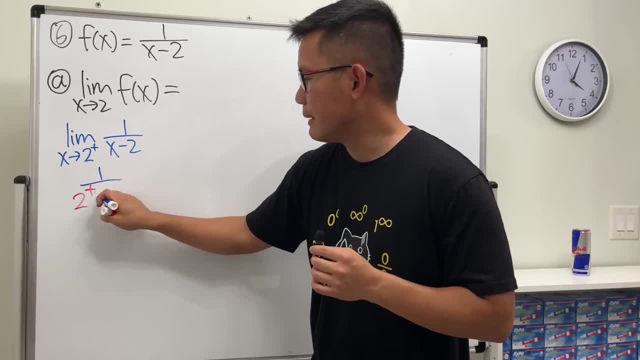 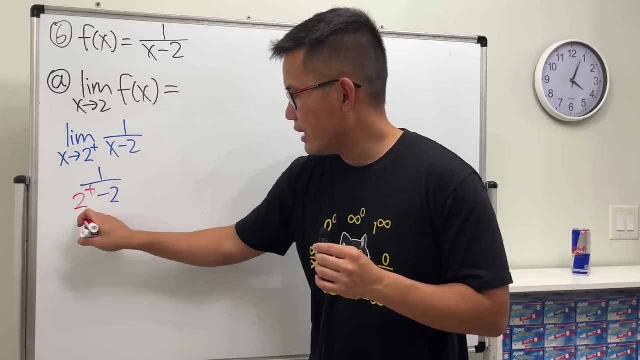 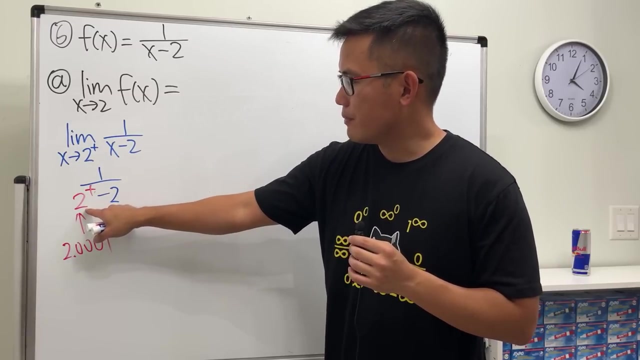 we are going to get one over two plus minus two. Two plus is just like a number slightly bigger than two. Just think about it like that And you can think about it as like 2.0001.. So earlier when we do like two minus two, not so much. 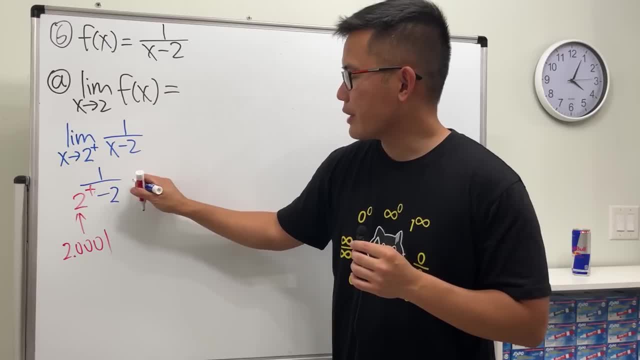 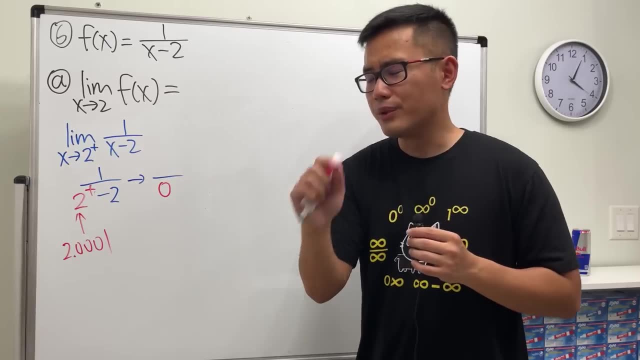 This is better: Two plus minus two- This right here is approaching zero. two minus two. This right here is approaching zero. Two minus two is zero, But this right here is a little bit more than two, So this zero is actually a little bit more than zero. 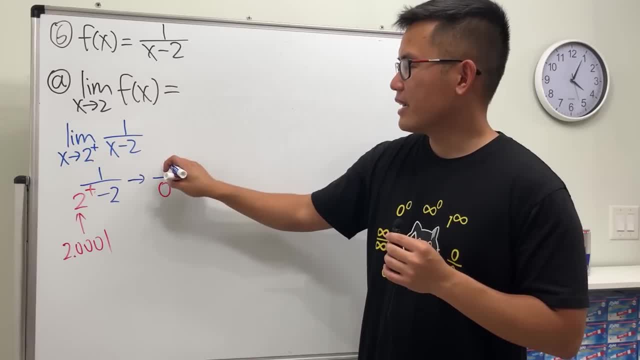 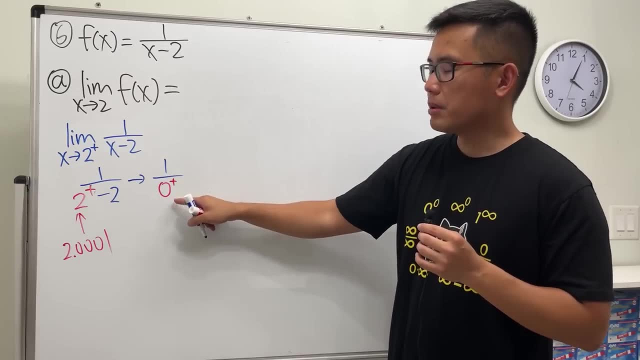 So this is technically zero plus, okay, And then on the top we still have the one, So we have one over zero plus, And when we have one over zero plus, when we're doing limits this right here, positive over positive, we get positive. 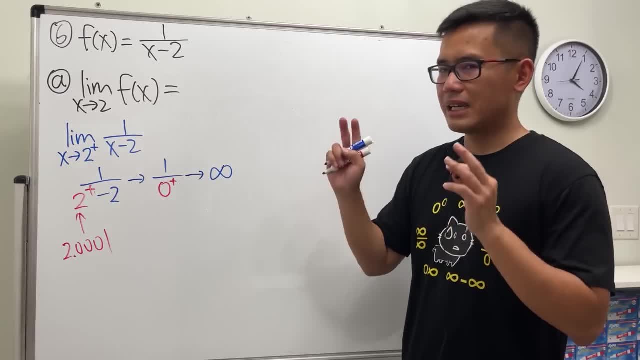 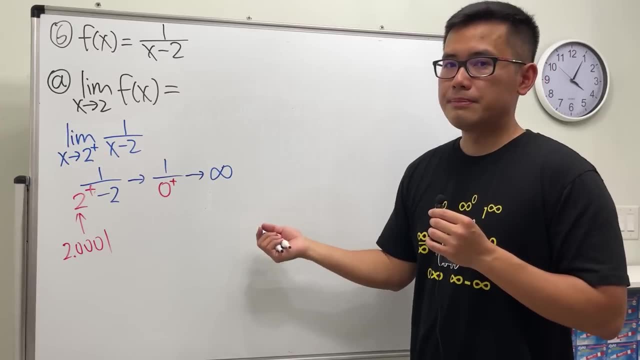 And then you get infinity. Whenever we are doing this kind of computation, if we have a zero plus or zero minus on the bottom, if the top is non-zero, then you are going to expect to get either positive infinity or negative infinity, And again just work out the sign. 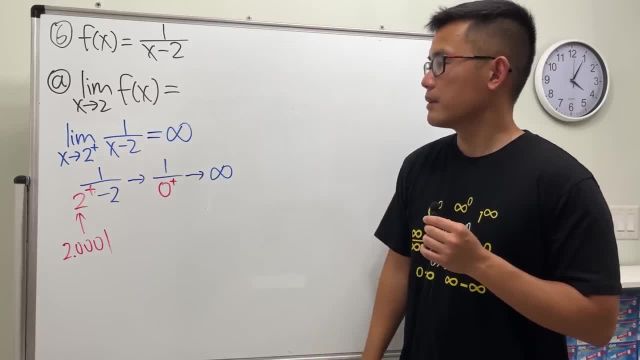 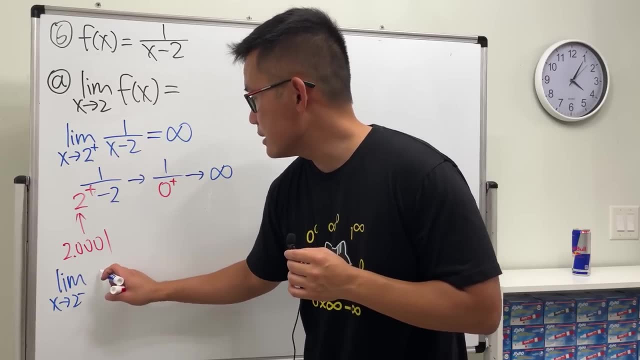 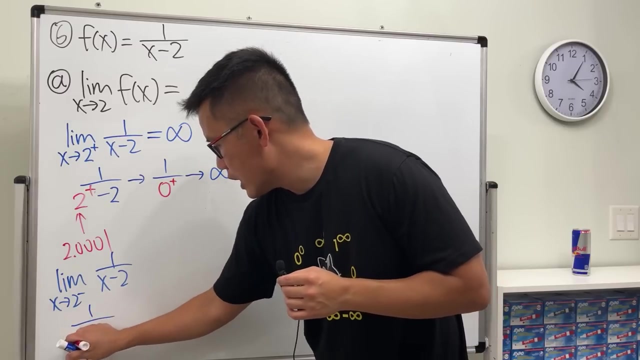 So this right here gives us positive infinity, okay. And then let's see if we have the limit as x approaching two minus, and then one over x minus two. Same thing. Put this right here now: We are getting one over two minus and minus two. 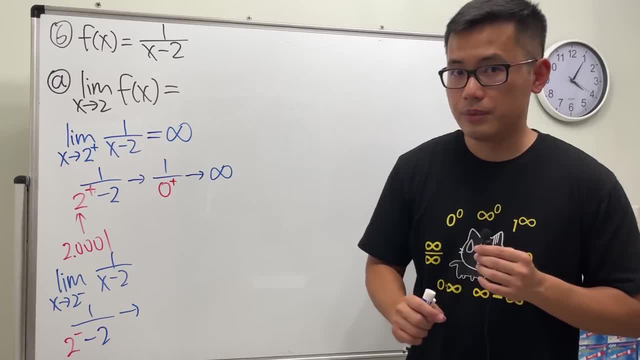 This: right here we are getting one over two minus and minus two. This right here we are getting one over two, minus and minus two. And this right here is a little bit less than two like 1.999.. This minus that, yes, it's like zero. 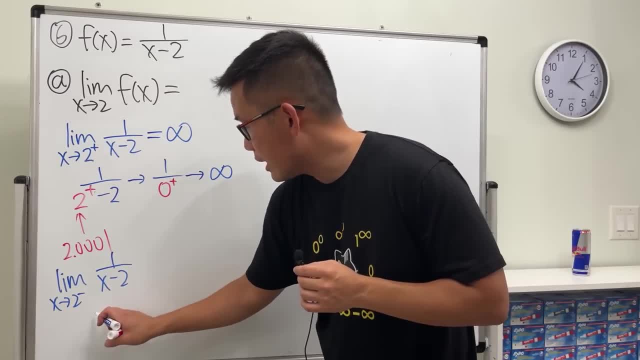 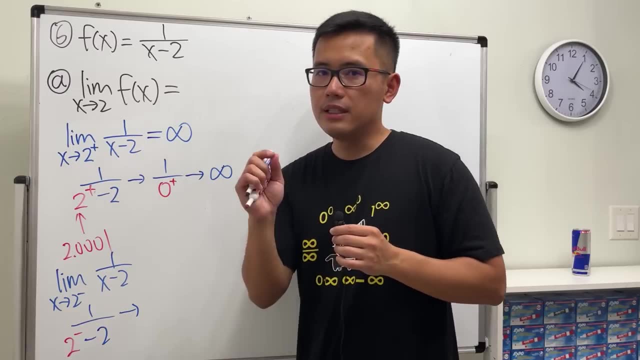 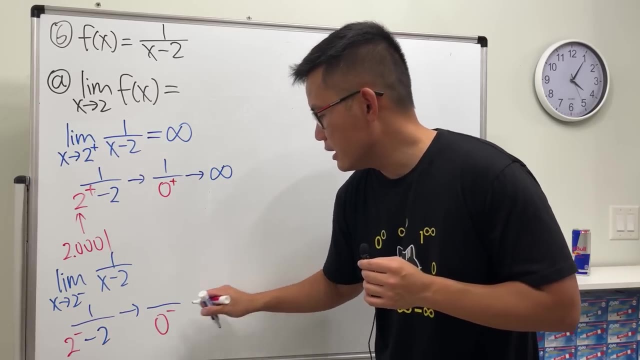 over x minus two, same thing. So if we do this right here now, we are getting one over two minus and minus two. This right here is a little bit less than two, like one point nine, nine, nine, This minus that, yes, it's like zero, but technically it's less than zero. 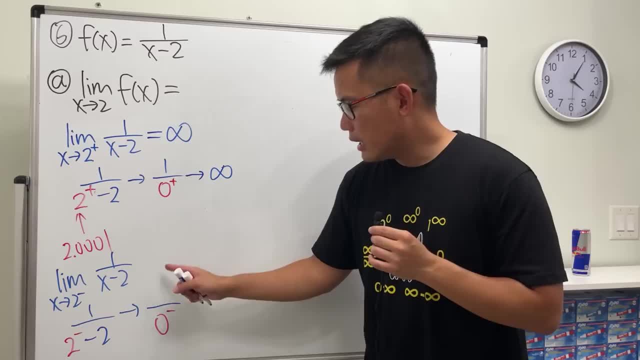 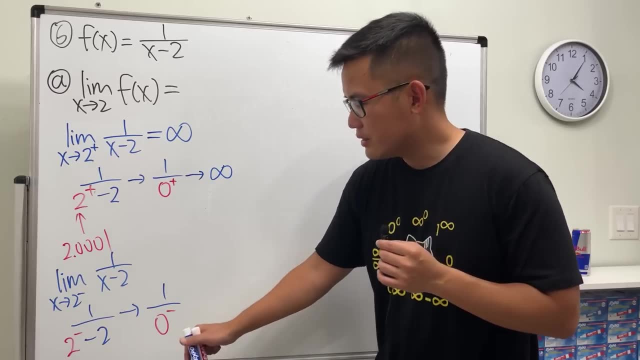 Just a little bit. That's why it's zero minus On the top is one One over zero minus. Zero minus is negative because, again, just think about this as one point: nine, nine, nine Minus two, we get negative small number. 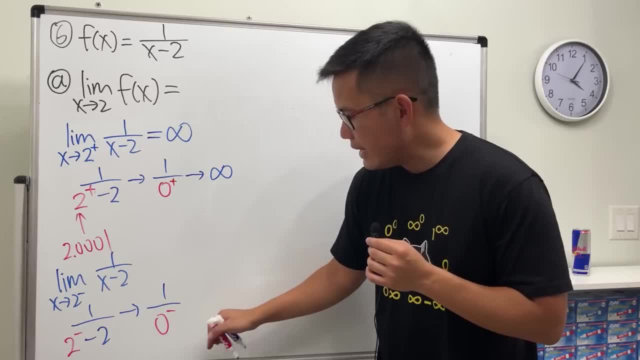 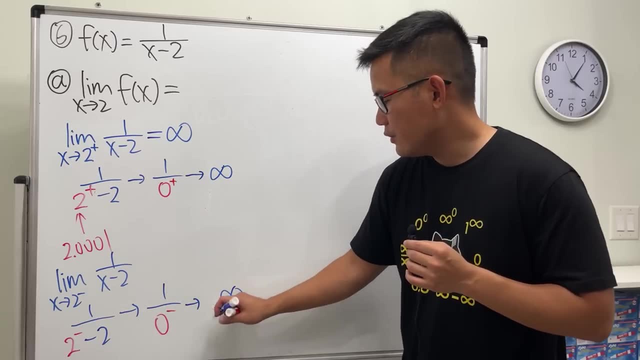 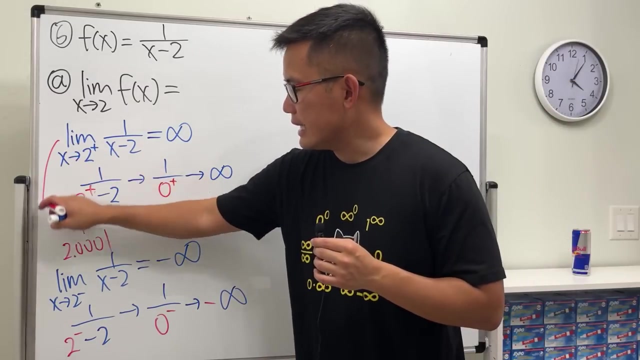 Zero minus is a negative. So we will end up with again: you have infinity, but just had to work out the sign Positive over negative. we have negative, So this right here gives us negative infinity. So you see this and that they are not equal. 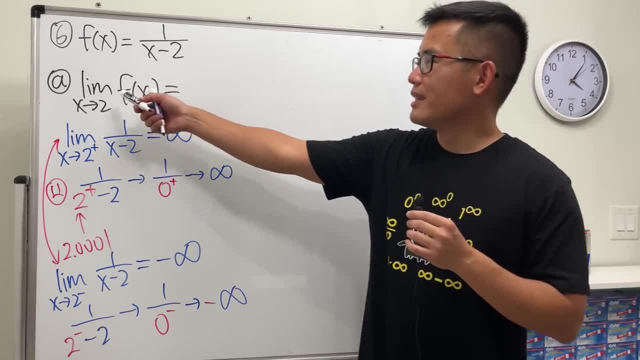 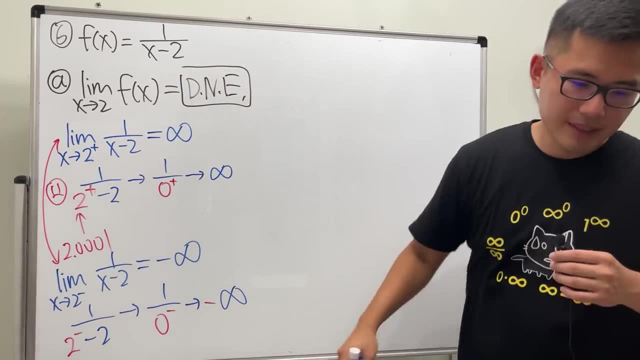 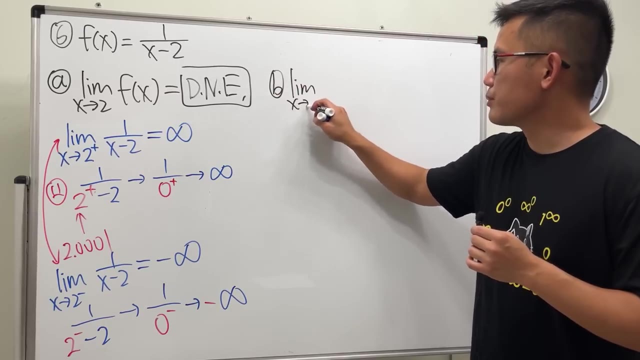 So this is like a sad face. That's why the answer for this right here is: does not exist, OK, does not exist, OK. part B: let's look at the limit as X approaching infinity of the function f of X. 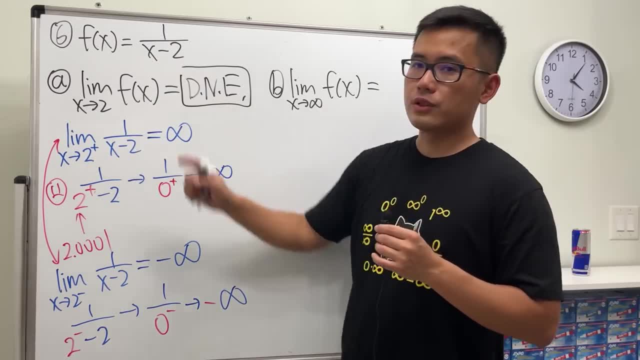 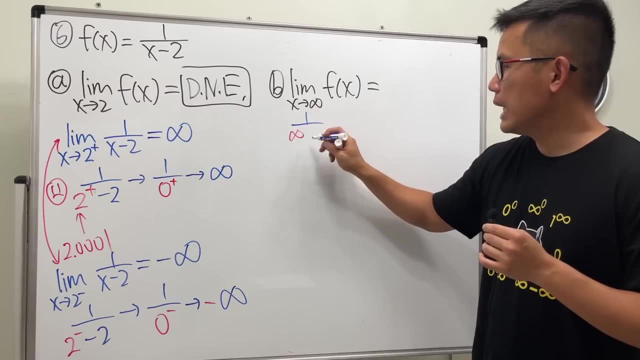 So for this one right here, let's see, if we put infinity to the function, then we are going to get one over one, over infinity minus two, And let's see if we can reason. Let's see if we can reason it out along the way. 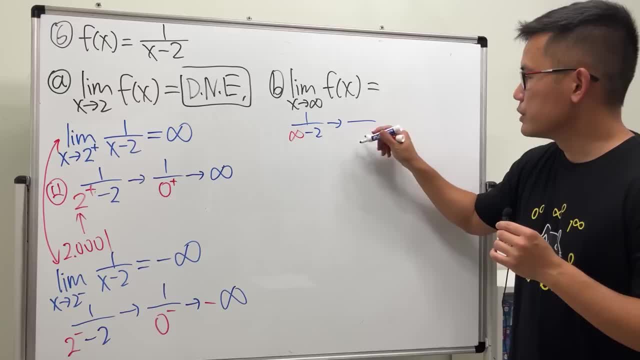 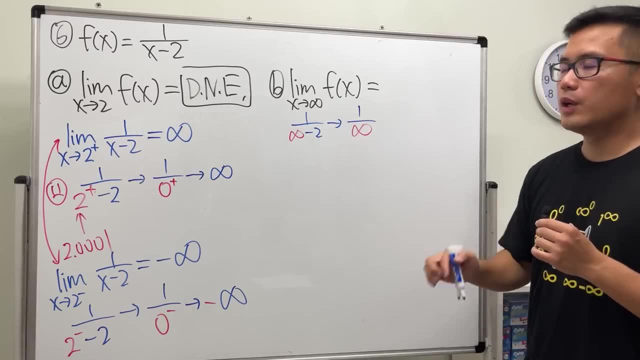 Infinity minus two is still infinity, So we still have the infinity on the bottom And we have a one on the top. If we have a finite number over infinity, guarantee we get zero right. One divided by infinity, yeah, approaches zero. 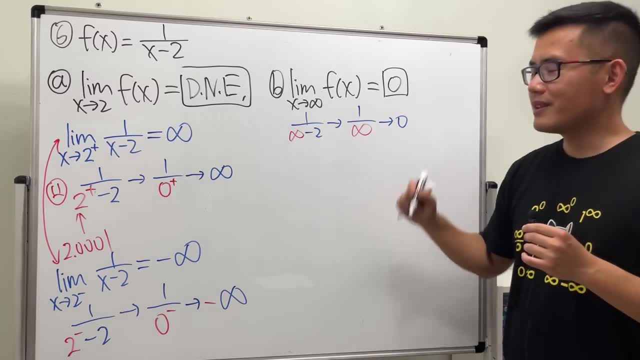 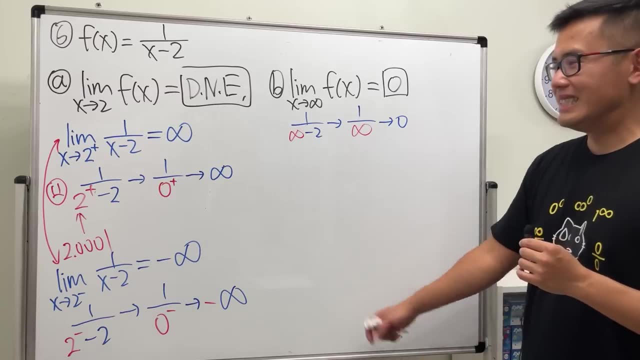 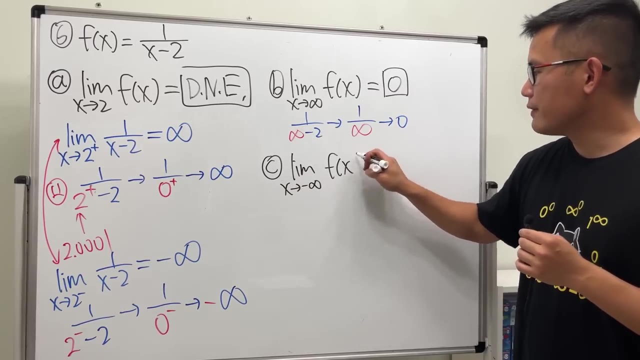 So the answer for this right here is just zero. Imagine one dollar, yeah, share with like one billion people, like 100 billion people. How much money is each person? And that kind of thing? Anyway, limit as X, approaching minus infinity of the function. 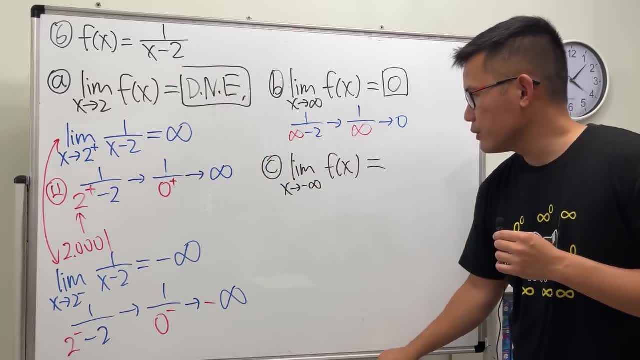 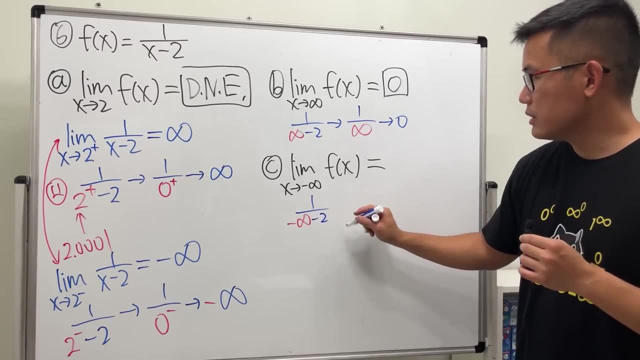 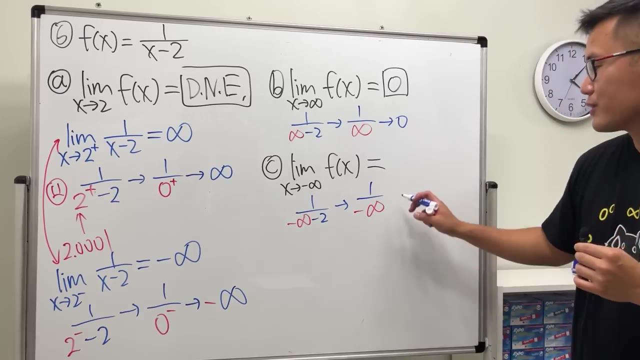 Put negative infinity into our function there. So we are looking at one over negative infinity, minus two, Minus infinity, minus two is still minus infinity And we have one over that right. But guess what? It's approaching zero. Don't say negative zero. 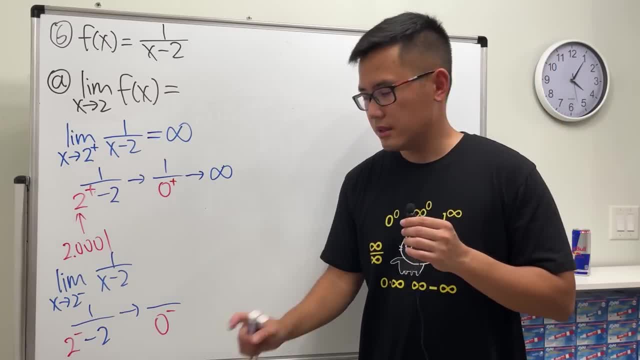 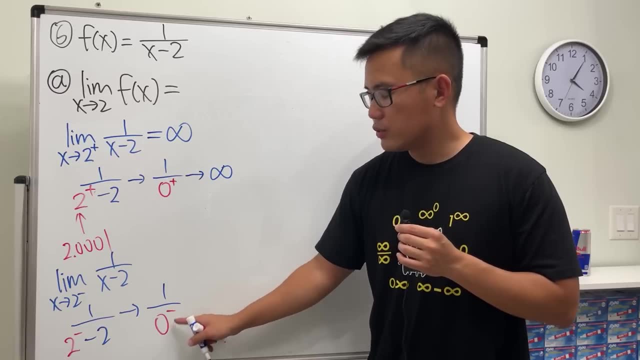 But technically it's less than zero, just a little bit. That's why it's zero minus On the top is one One over zero minus. Zero minus is negative Because again, just think about this as 1.999 minus two. 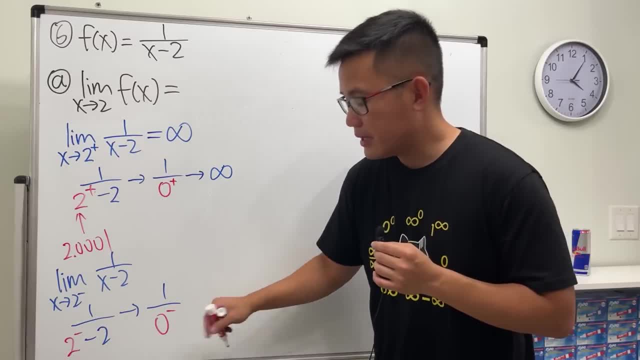 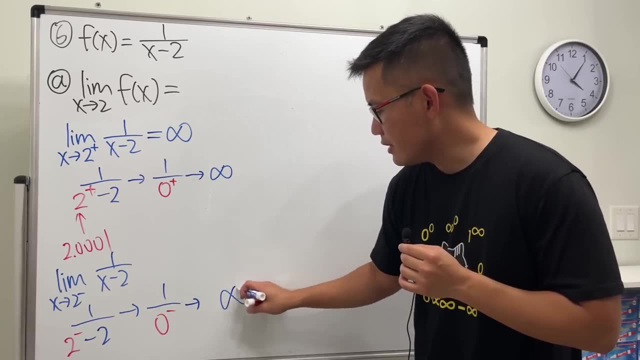 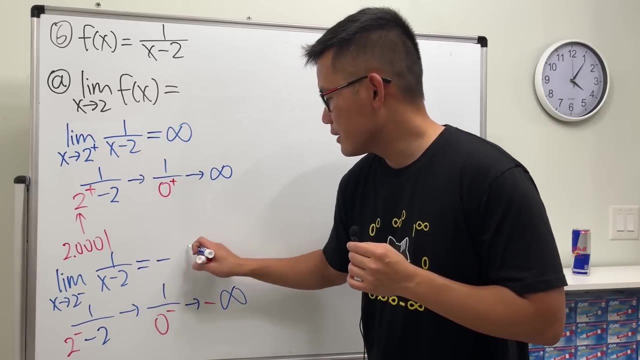 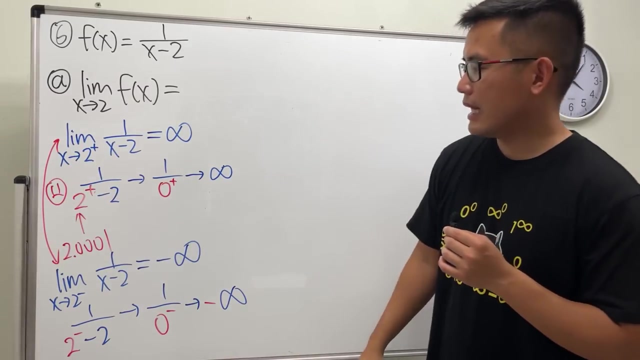 We get a negative small number. Zero minus is a negative. so we will end up with again: you have infinity by just how to work out the sign positive over negative. we have negative, so this right here gives us negative infinity. so you see this, and that they are not equal, so that this is like a sad face. that's why the answer for 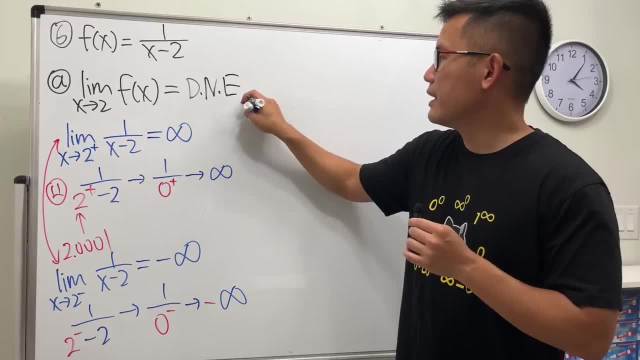 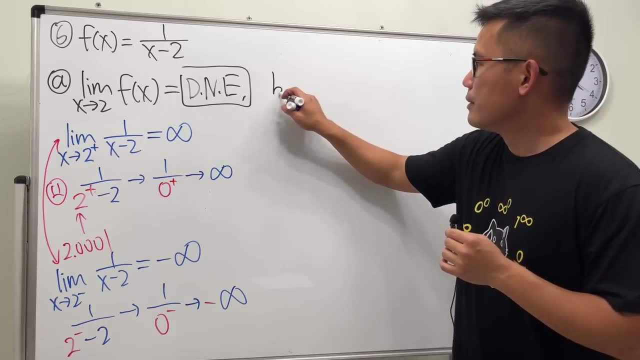 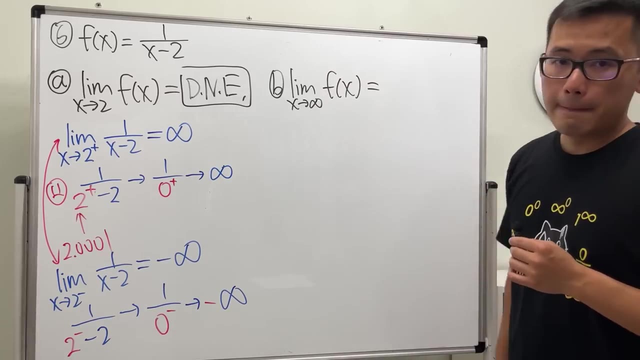 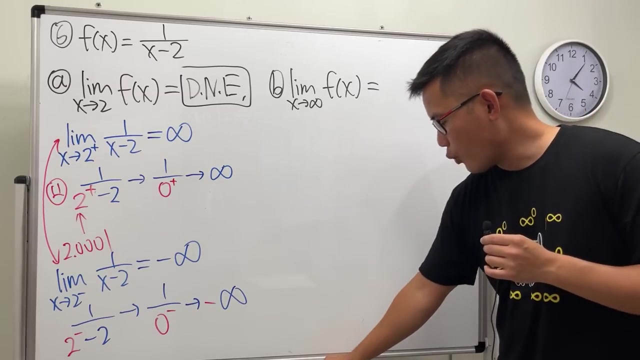 this right here is: does not exist, okay, does not exist, okay. part b: let's look at the limit as x approaching infinity of the function f of x. so for this one right here, let's see: if we put infinity to the function, then we are going to get 1 over 1 over infinity minus 2.. and 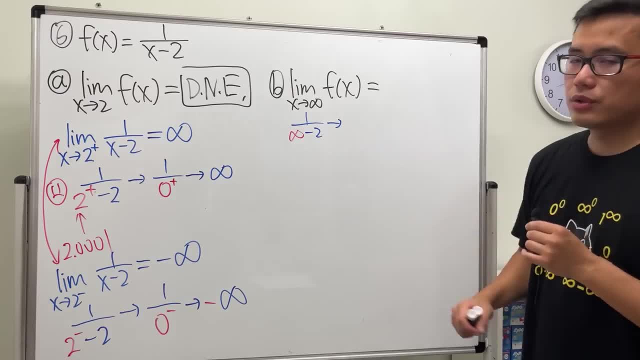 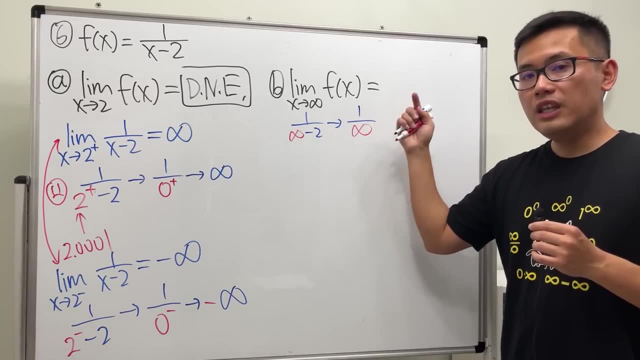 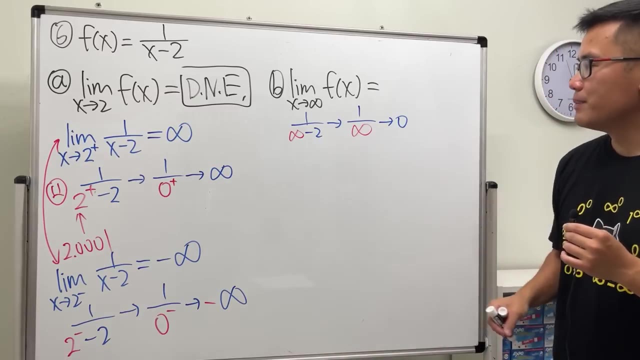 that's see if we can reason it out along the way. infinity minus two is still infinity, so we still have the infinity on the bottom and we have a one on the top. if we have a finite number over infinity, guarantee we get zero, right, one divided by infinity. yeah, the approach is zero. so the answer: 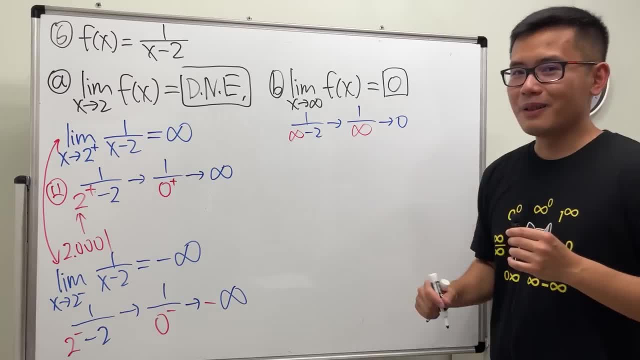 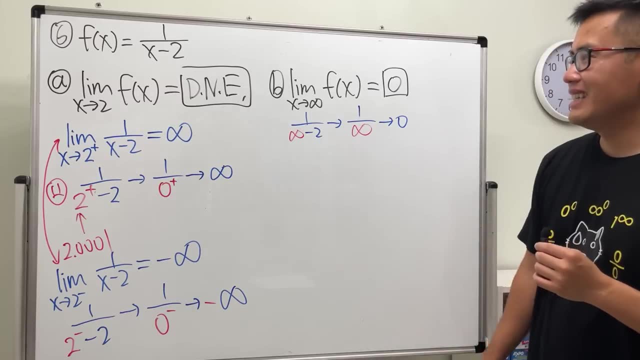 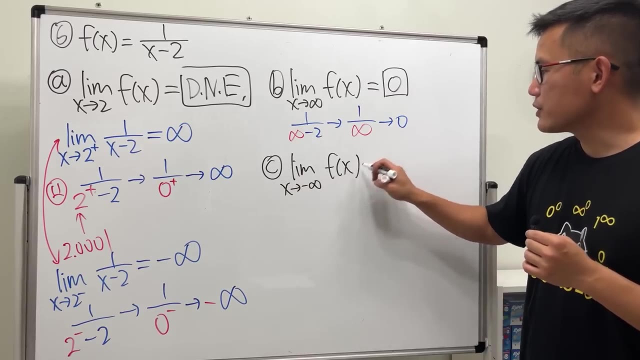 for this right here is just zero. imagine one dollar, yeah, share with like one billion people, like 100 billion people. how much money is each person going to get? and that kind of thing anyway, limit as x approaching minus infinity of the function. put negative infinity into our function. 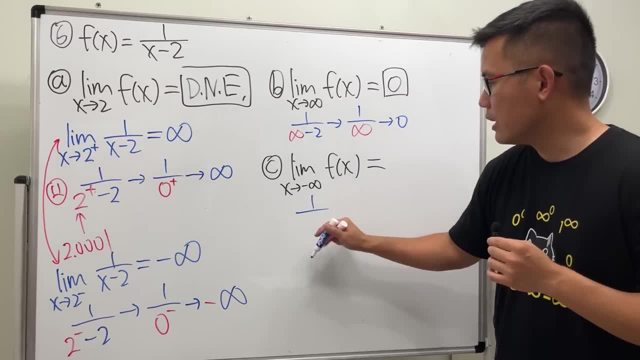 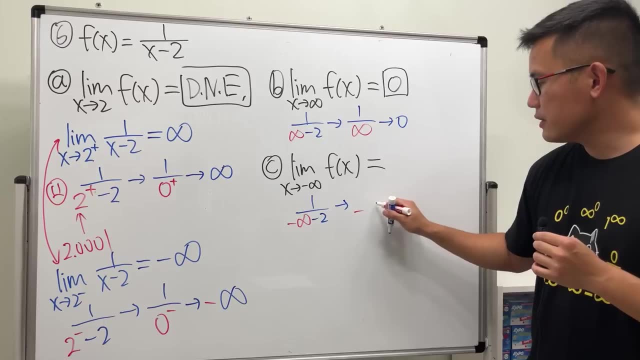 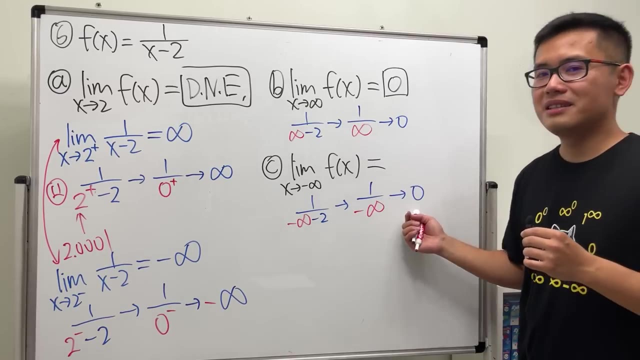 there. so we are looking at one over negative infinity minus two. minus infinity minus two is still minus infinity, and we have one over that right, but guess what? it's approaching zero. two say negative zero, it's the same as zero. yeah, so that's why, when you have a non-negative number, 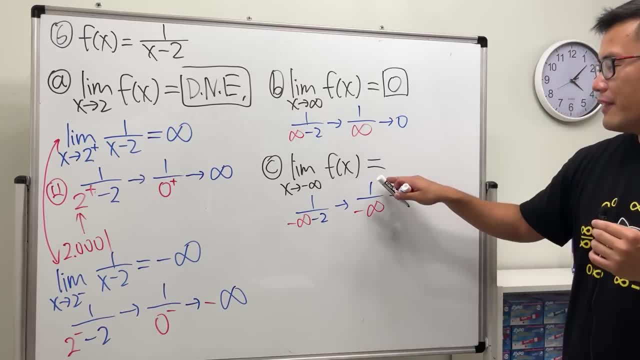 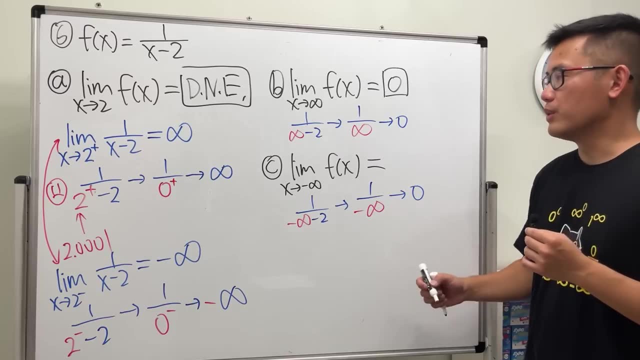 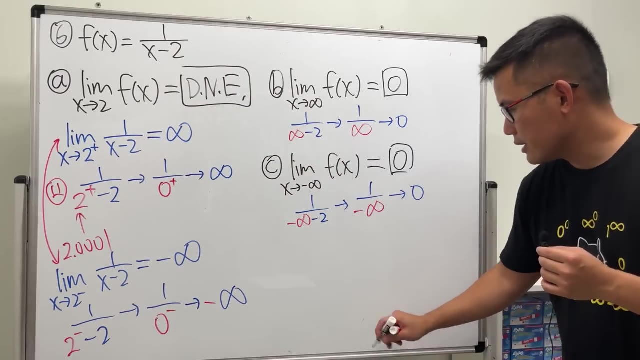 It's the same as zero. So that's why, when you have a non-negative number- sorry, when we have a non, when we have a finite number over infinity, we get zero. So this right here is just zero down here. Now let me show you guys the graph of this. 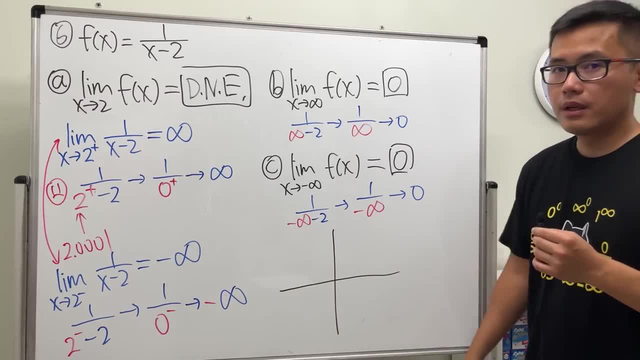 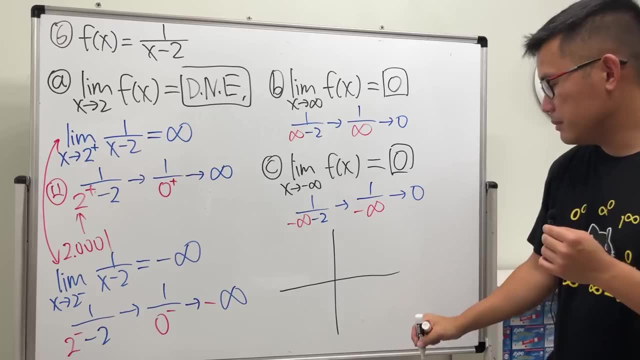 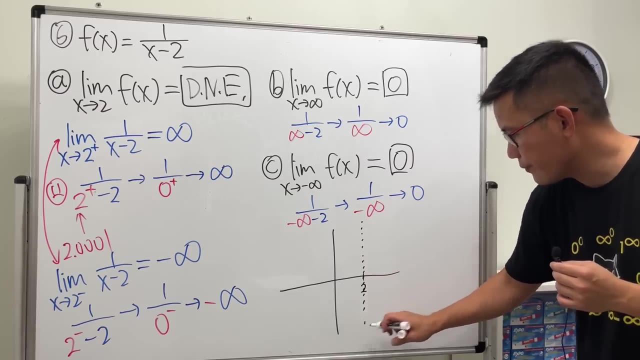 If we have one over X minus two, it's just a one over X, which is like this, like that. But because it's a X minus two on the bottom, we actually have a vertical as the right here at two And we have a vertical as the top, like so. 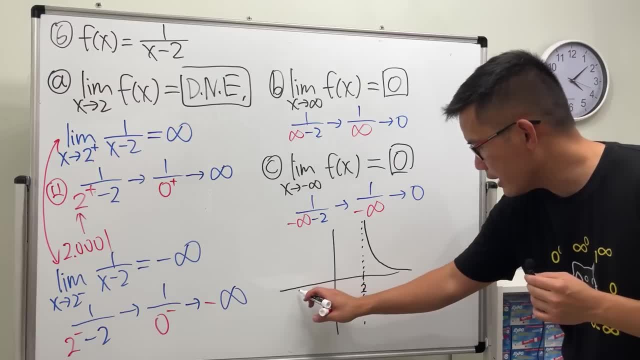 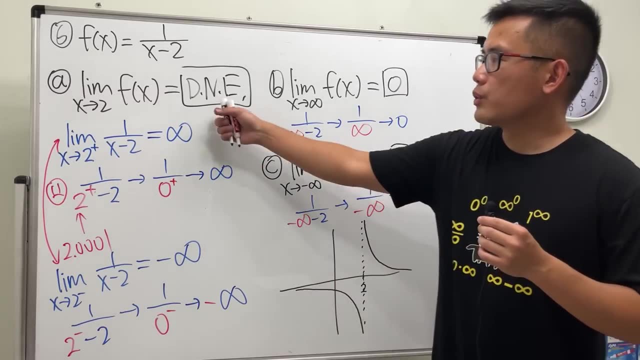 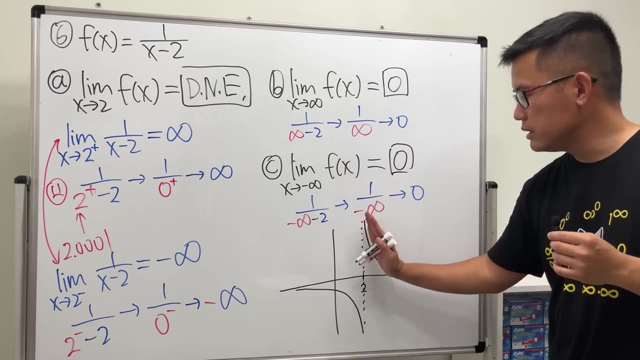 And then the curve looks like this, like that. So if you have this picture in your mind earlier, this question will be much easier, because you can see that the limit as X approaching to two from the right, this right here, is positive infinity. 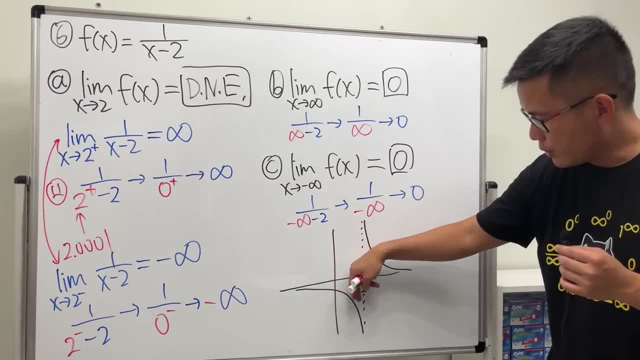 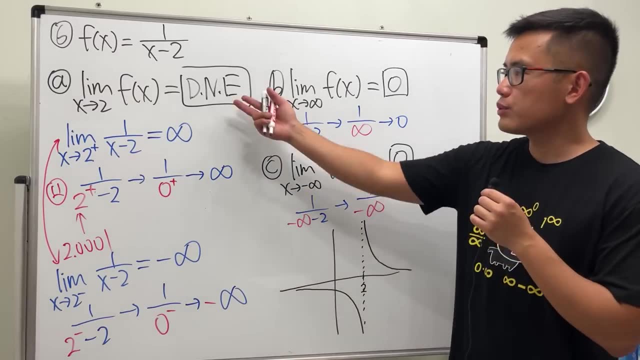 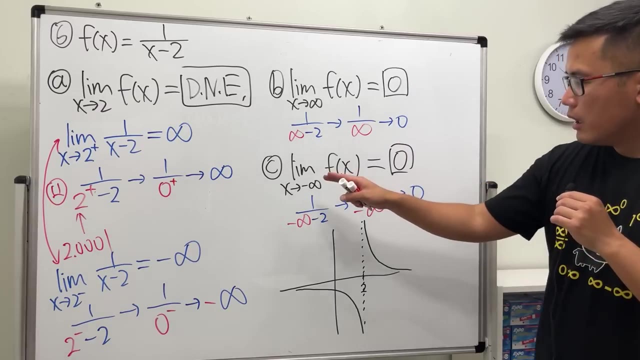 as we mentioned earlier. and then you get negative infinity when we go from the negative side, right, So that's that. And then they are not approaching to the same Y-value. That's why this doesn't exist. And then, when X is approaching infinity, the Y-value is approaching zero. 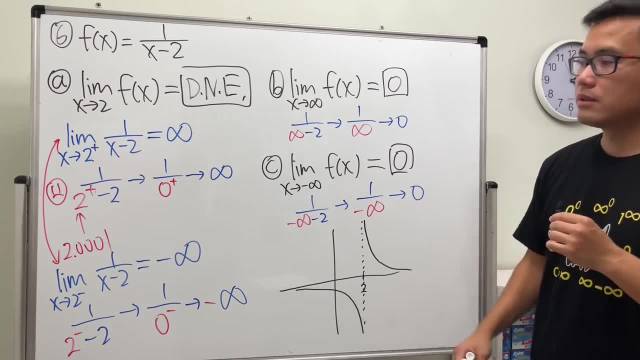 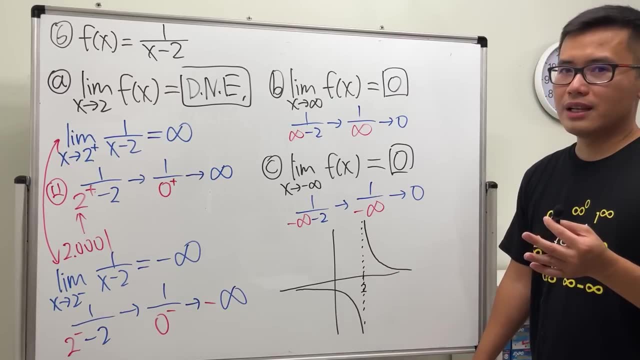 The Y-value is approaching zero when X is approaching negative zero. So yeah, so this is number six, So note your graphs. I'm pretty sure, if you are taking your Calc 1 class, or maybe pre-calc, if you are watching this for your pre-calculus class. 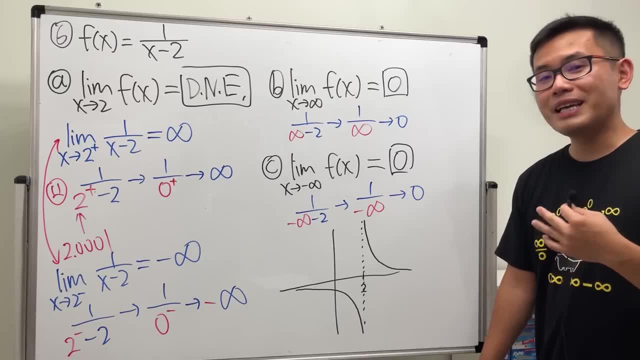 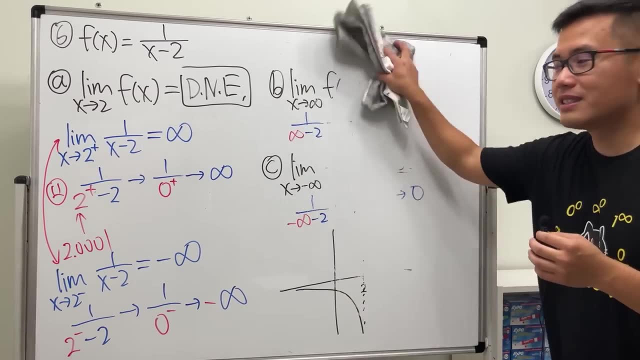 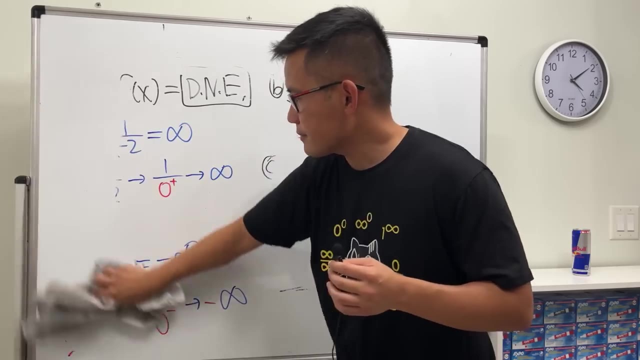 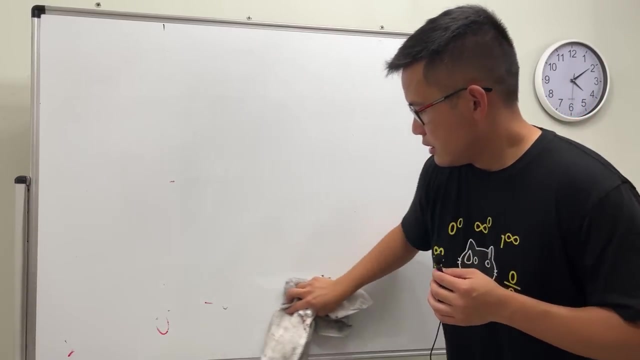 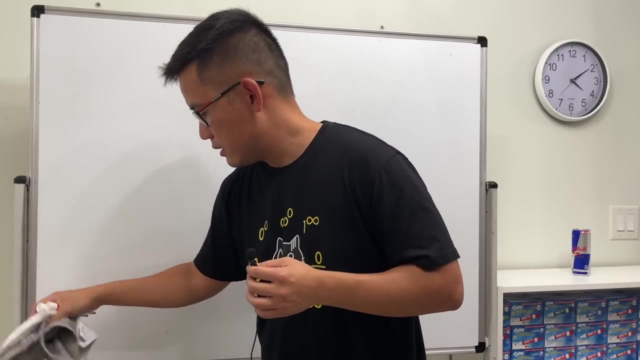 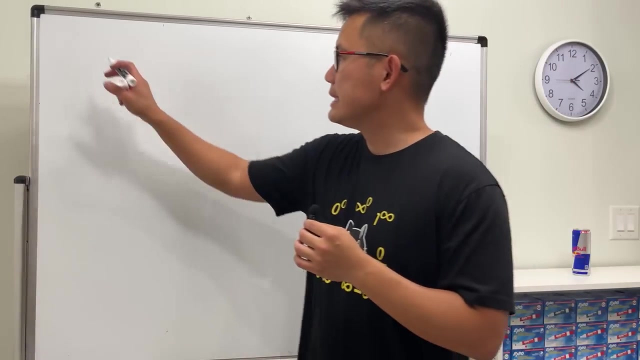 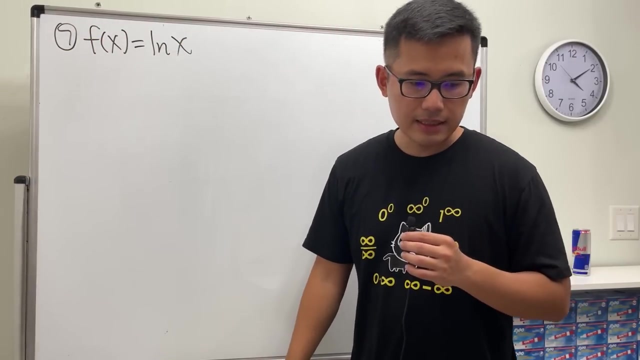 your teacher will, would like you to know the graphs of this: basic functions, the rational functions, the square root functions, and then the other ones that I am about to mention. All right, So number seven, our function is natural log of X. 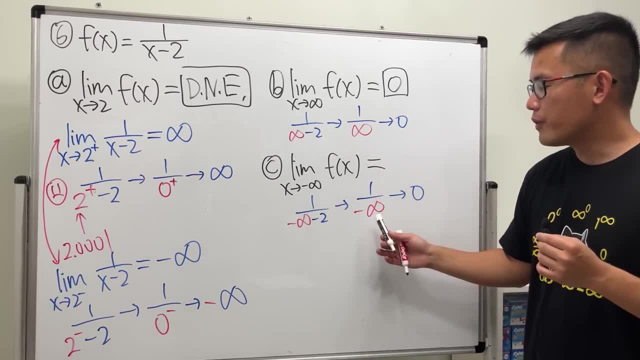 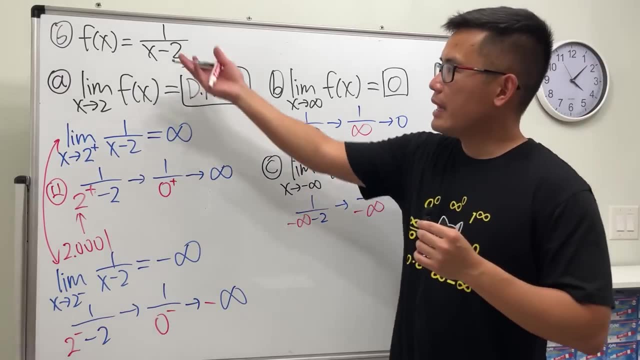 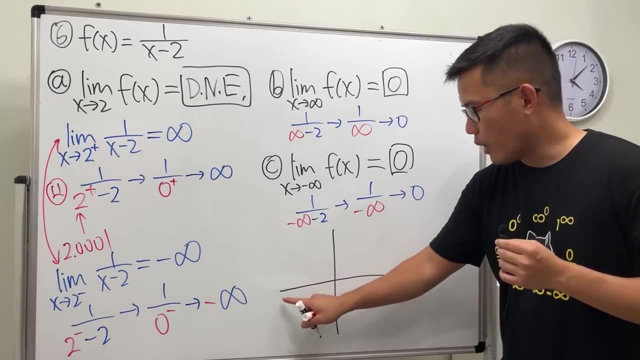 sorry. when we have a non, when we have a finite number over infinity, we get zero. so this right here is just zero down here. now let me show you guys the graph for this. if we have one over x minus two, it's just like one over x, which is like this, like that. but because it's a x minus 2 on the 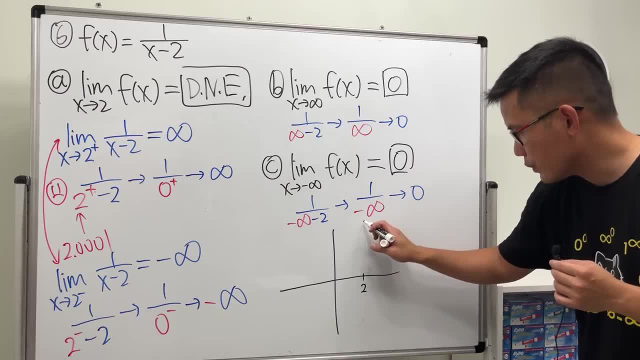 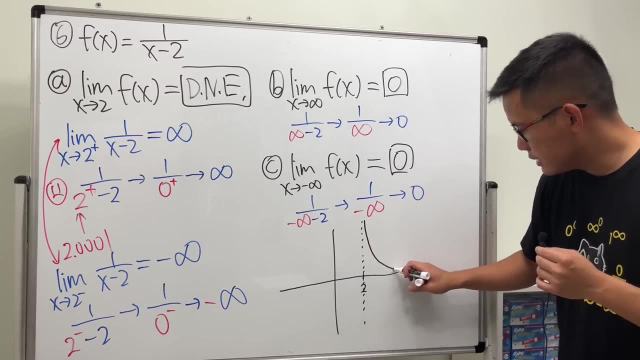 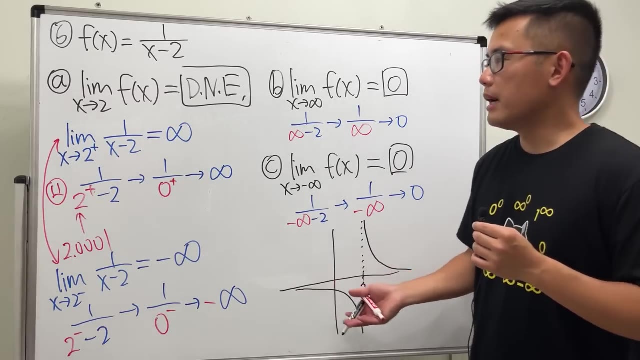 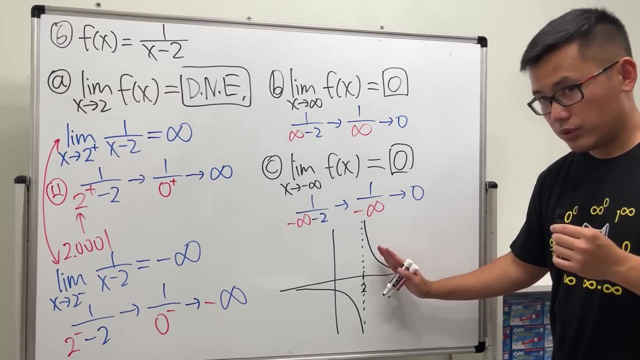 bottom. we actually have a vertical stop right here at two. then we have a vertical acetone like so, and then the curve looks like this, like that. so if you have this picture in your mind earlier, this question will be much easier, because you can see that the limit as x approaching to two from the right, this 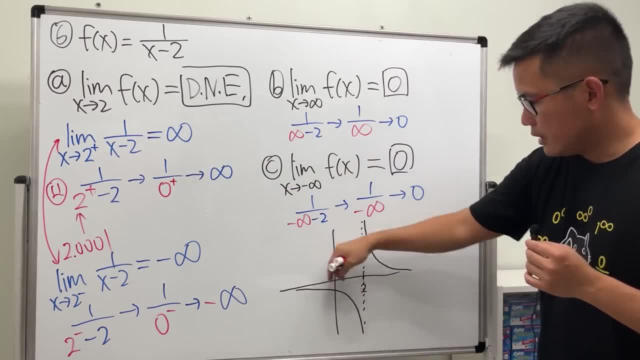 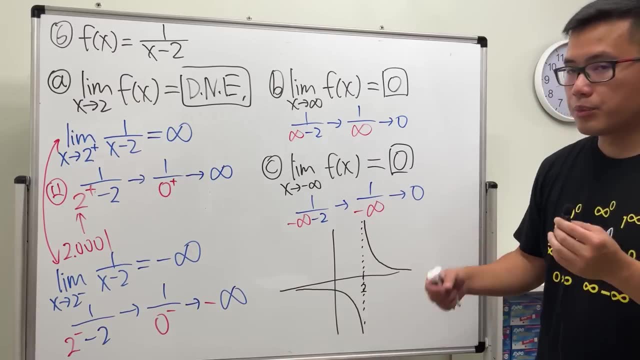 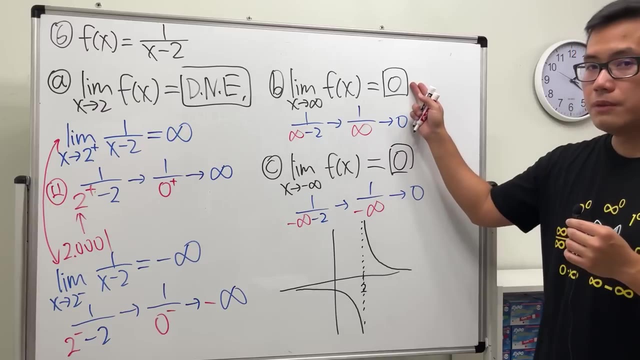 right here is positive infinity, as we mentioned earlier, and then you get negative infinity when we go from the negative side, right, so that's that. and then they are not approaching to the same y value. that's why this doesn't exist. and then, when x is approaching infinity, the y4 is approaching zero. 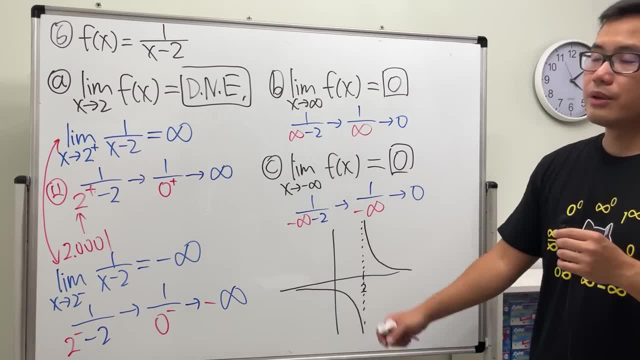 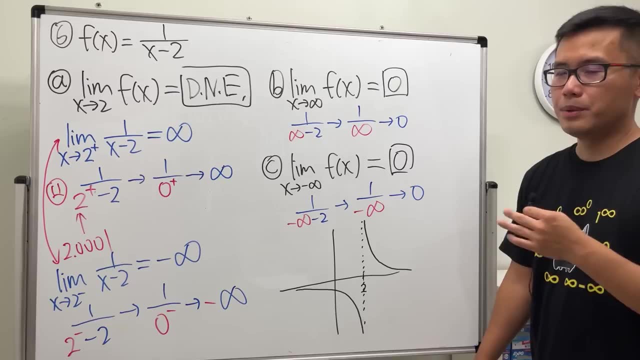 the y file is approaching zero when x is approaching negative zero. so yeah, so this is number six, so note your graphs. i'm pretty sure if you are taking your carbon class or maybe pre-calc, if you are watching this for your pre-calculus class- uh, your teachers will. would like you to know the graphs of this. basic functions like the: 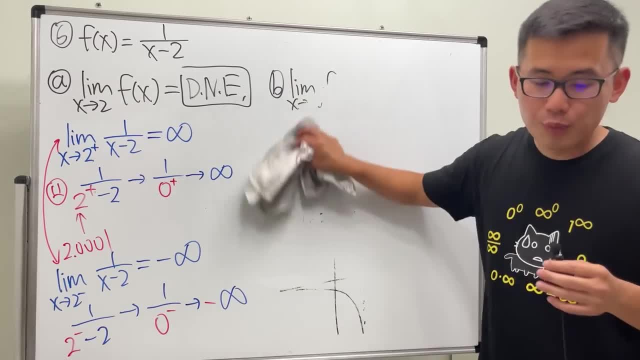 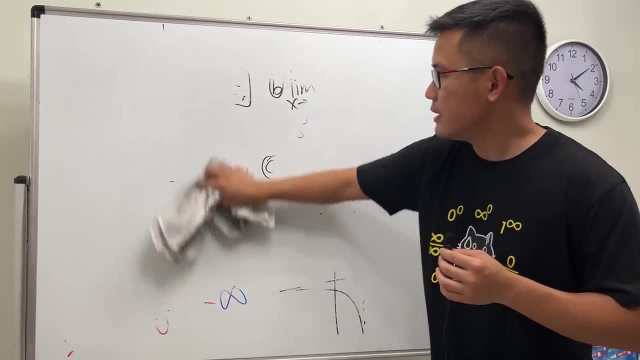 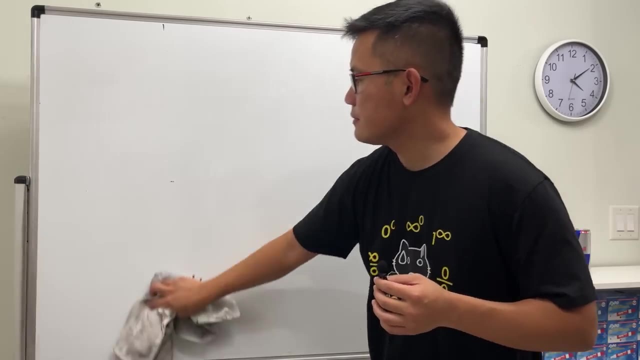 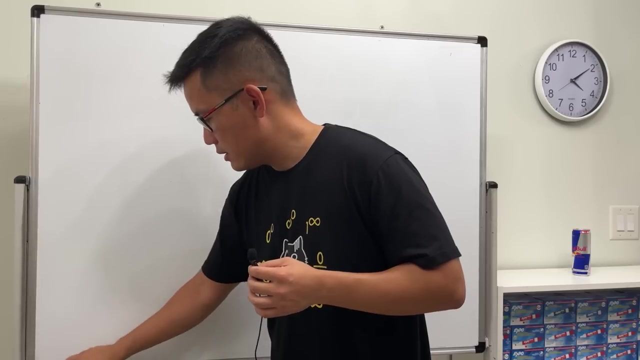 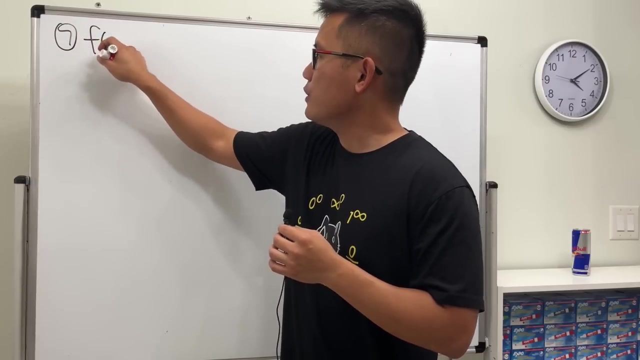 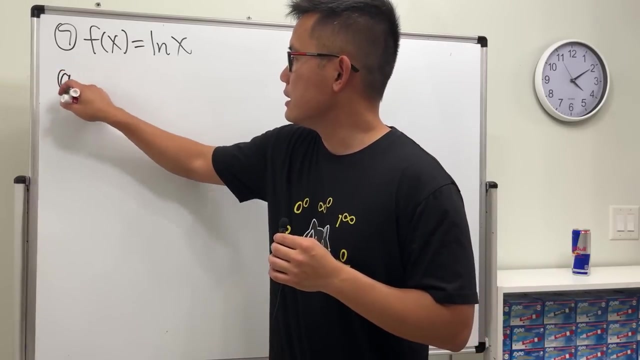 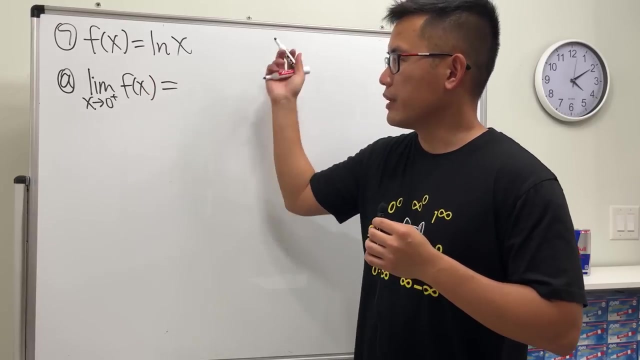 rational functions, the square root functions, and then the other ones that i am about to mention. right, so number six. i open this function here before i write it down. alright, so number seven: our function is natural log of x. so Part eight, let's see, we want the limit. 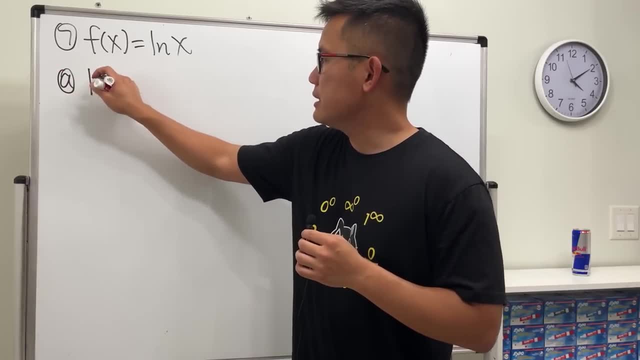 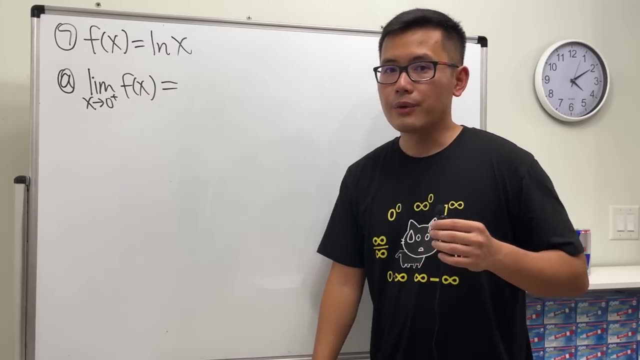 So part A, let's see. We want the limit as X approaching zero plus of the function L and X. pretty much, So let's see what will we get when we have zero plus inside here. Well, let me tell you, it looks like this right. 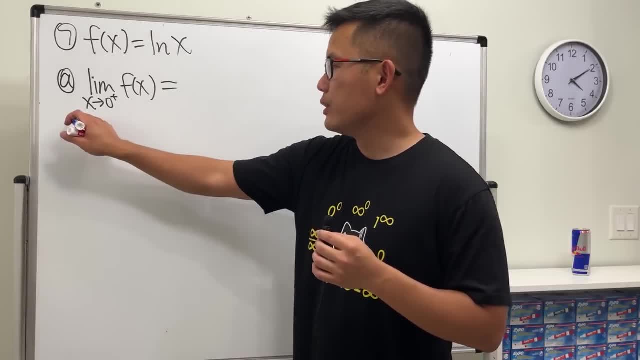 as x approaching zero plus of the functionszyst km of ln of x. pretty much. so let's see what we get when we have SU S3—1,0 for smX, b1,0 for l1x of a NAS variant, zero plus inside here. well, let me tell you, it looks like this, right, if you just want to plug. 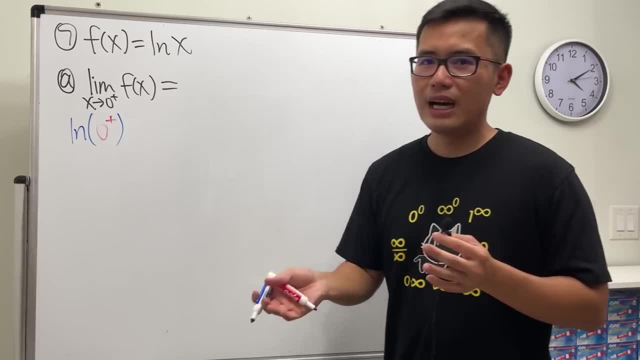 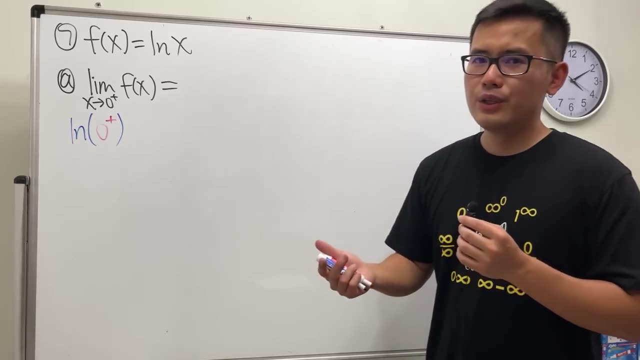 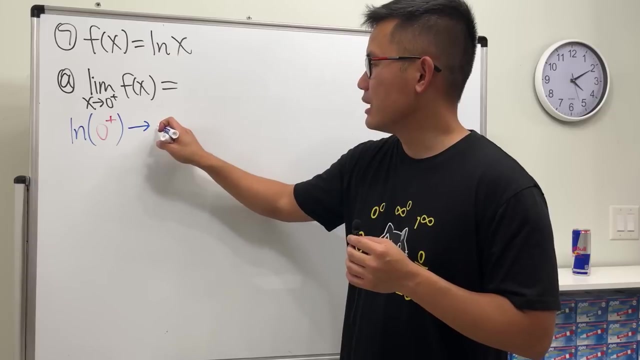 If you just want to plug in, and then, kind of recently, I will do computation. Here's the deal. If you have ln of zero plus, in fact, you will have to know the graph in order to actually see what the answer is. I will tell you, though: the answer for this right here is negative infinity. 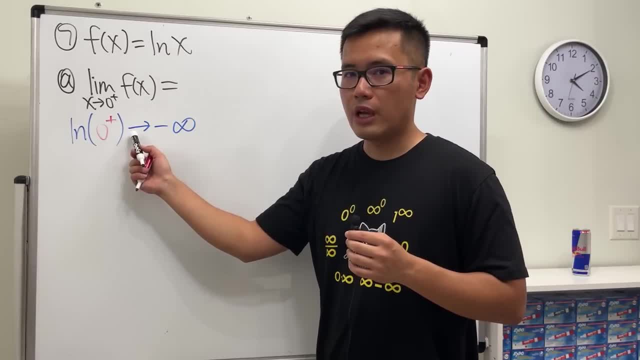 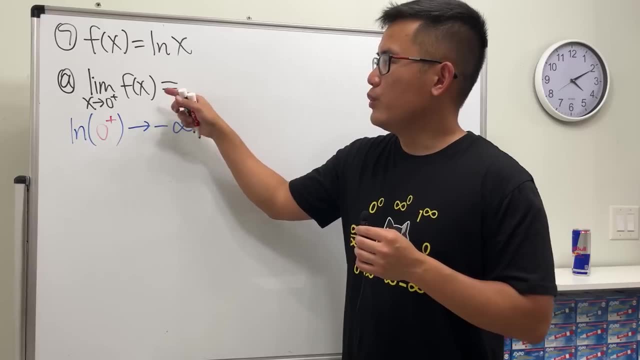 The approach is negative infinity. And notice that how I have been drawing arrows when I do this kind of computations, because arrow means approach. But when we have the limit and then we put equal, because the limit has that approach already, We are trying to answer limits equal to whatever. 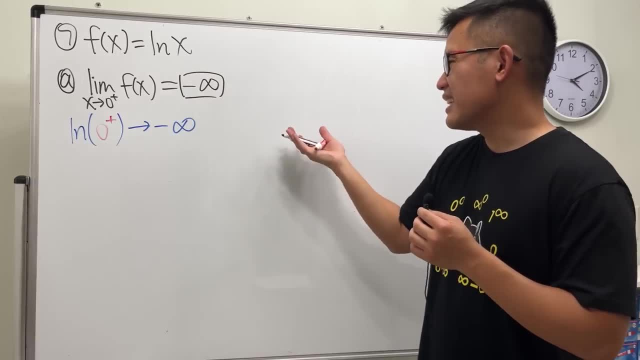 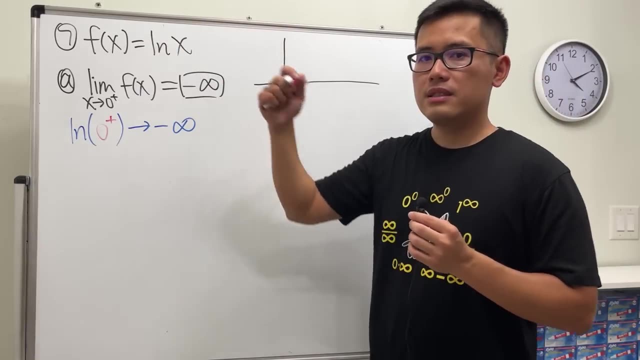 But anyway, though, the answer is negative infinity right here, And, as I said, I think it would be much better if I just give you guys a graph right now to make sense of this ln of X. one of the functions that you definitely will have to know looks like this: 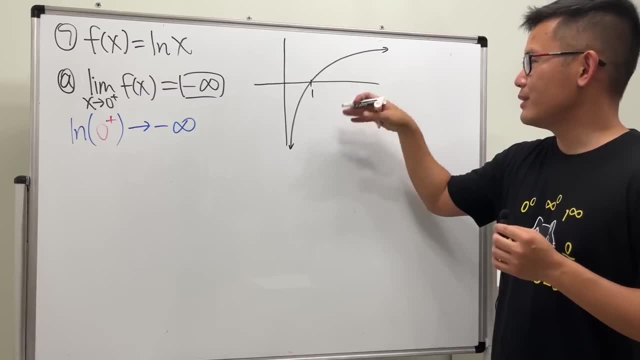 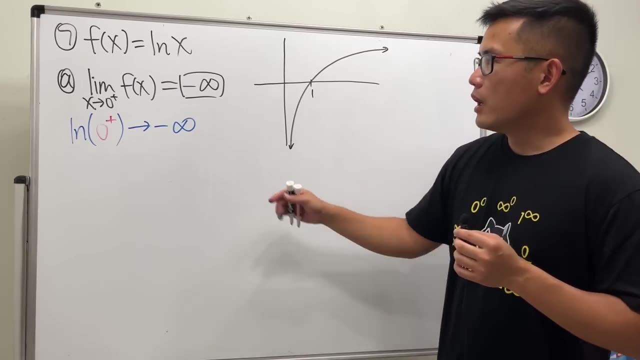 Yeah, some effect for the wing, Anyway, one and all that. So when X is approaching zero from the right hand side you see the function is going straight down and the ln X. it only makes sense when X is greater than zero. 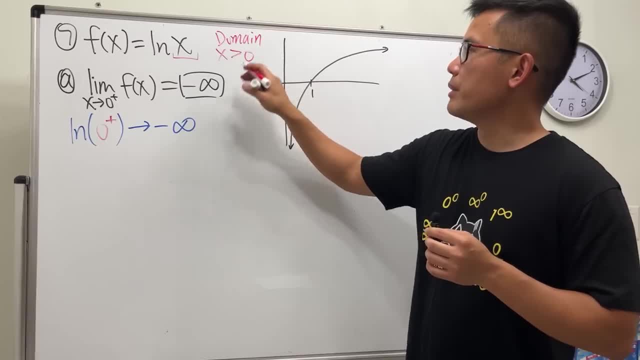 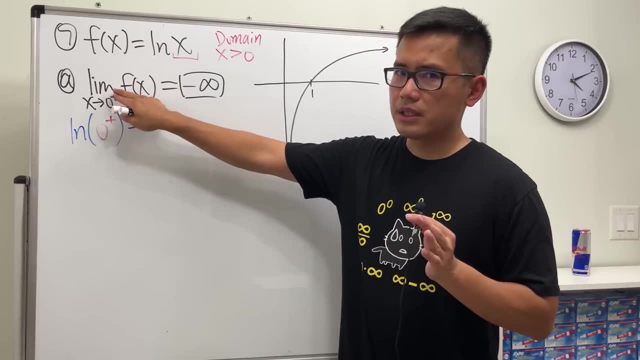 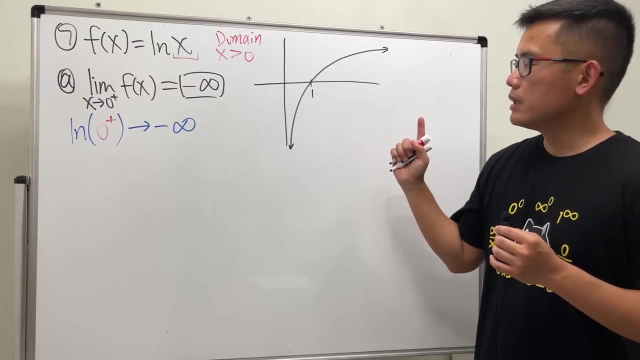 This is the domain of the function, Domain of the ln. the inside has to be greater than zero. That's why X approaching just zero wouldn't make sense. X approaching zero minus wouldn't make sense either. So that, and then let me see. 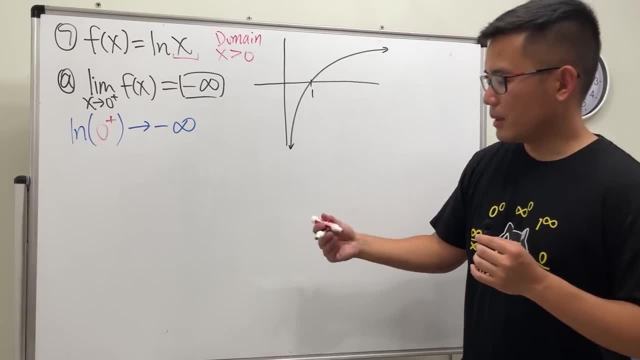 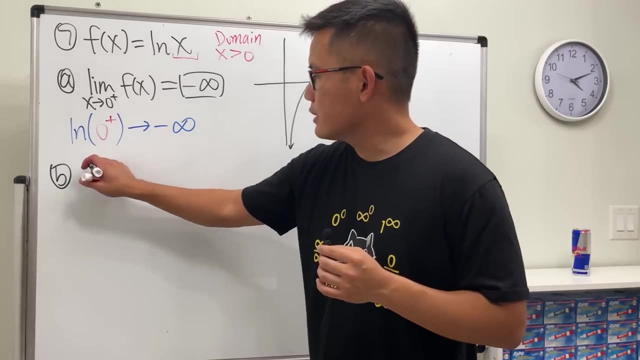 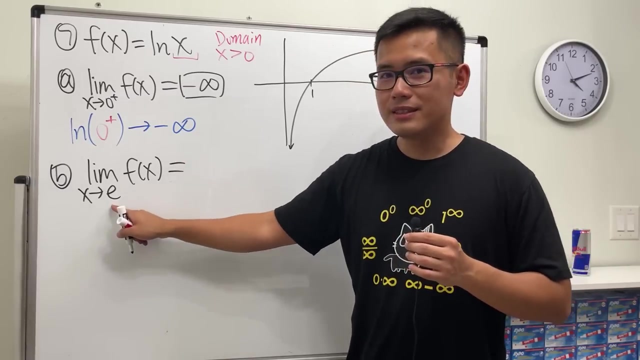 What else do I have I don't want to mention. Yeah, that's all. moving to the next one, B. OK, next one: limit as X approaching E of the function. When X is approaching E, we can put E into ln X and guess what? 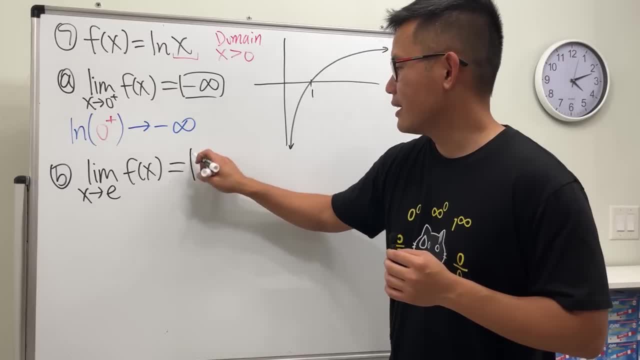 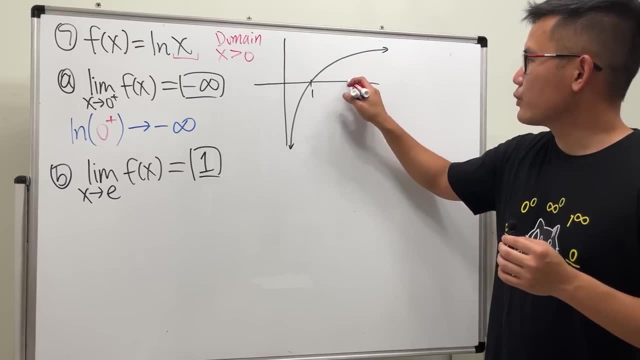 ln E is just equal to one. So the answer is just one. In fact, E is about like 2.718, right? So let's say E is about right here. When we put E into the ln function, you see how the function is nice and continuous. 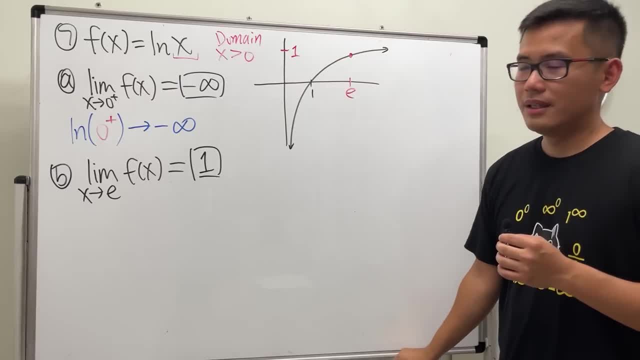 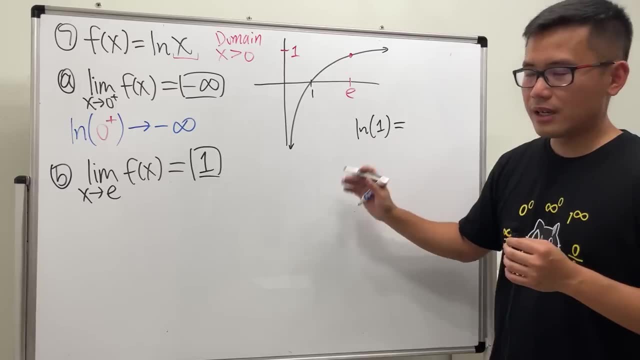 And the y-foil here is one. Yeah, that's it. So some of the values that you definitely have to know: ln one- this is not limit, It's just a regular computation. ln one is zero and then ln E is one. 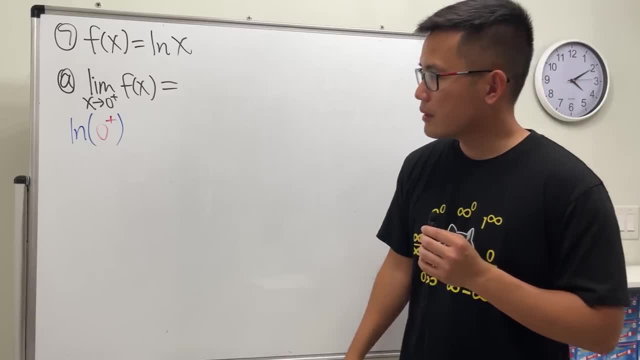 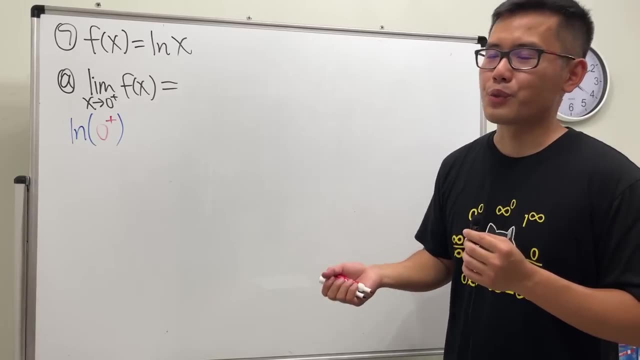 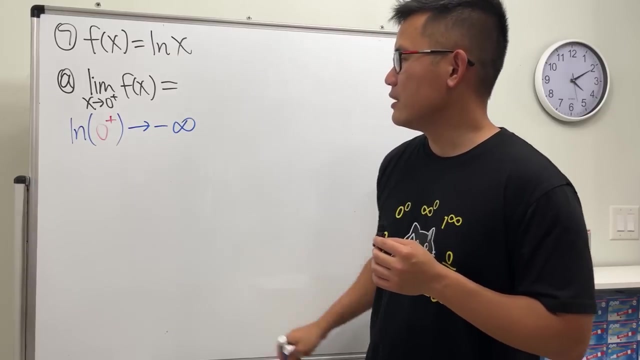 in and then, kind of recently, i will do computation. here's the deal: if you have ln of 0 plus, in fact, you will have to know the graph in order to actually see what the answer is. i will tell you, though. the answer for this right here is negative: infinity. the approach is negative. 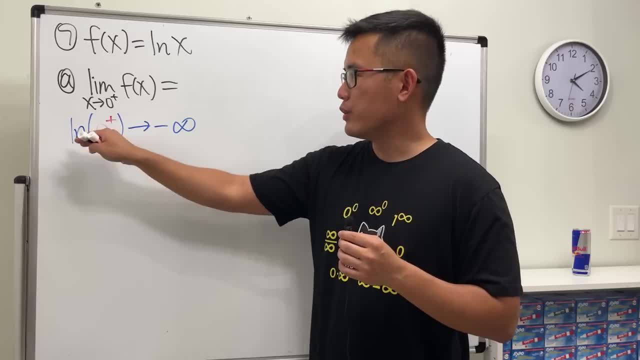 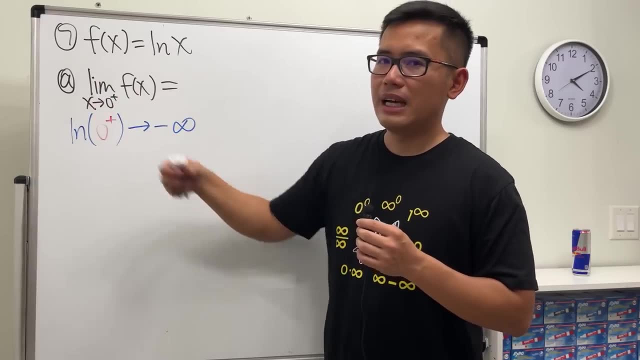 infinity, and notice that how i have been drawing arrows when i do this kind of computations, because error means approach, but when we have the limit and then we could equal because the limit has that approach already, we are trying to answer limits equal to whatever. but anyway, though, the 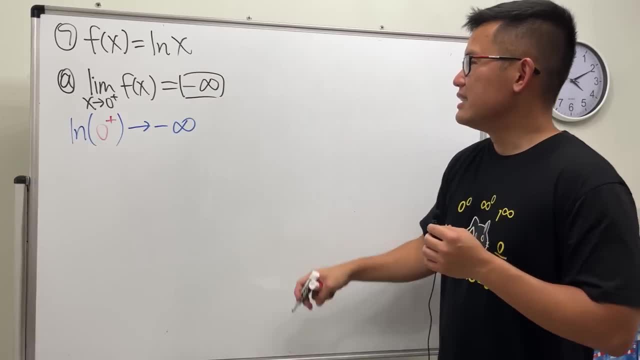 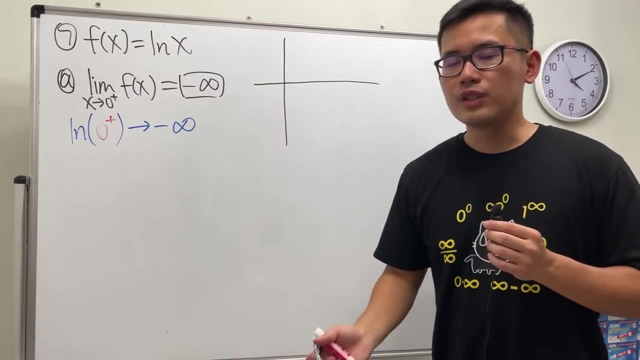 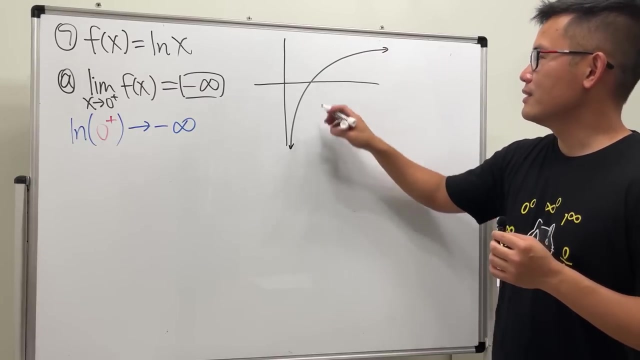 answer is negative infinity right here. and, as i said, i think it would be much better if i just give you guys a graph right now to make sense of this. ln x, one of the functions that you definitely will have to know, looks like this: yeah, some effect for the wing, huh, anyway, one and all that. 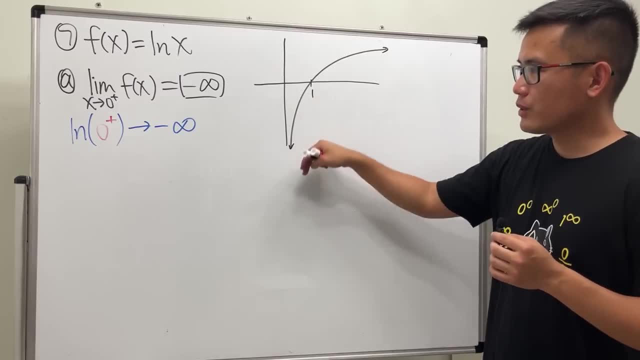 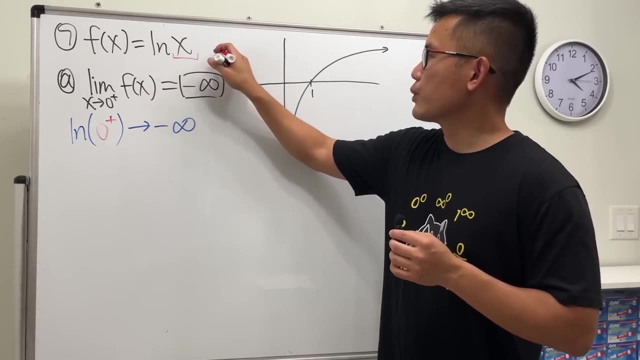 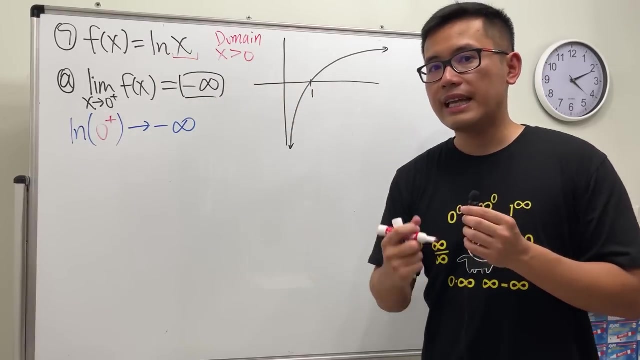 so when x is approaching zero, from the right hand side you see the function is going straight down and uh, ln, x. it only makes sense when x is greater than zero. this is the domain of the function, right domain of the ln. the inside has to be greater than zero. that's why x approaching 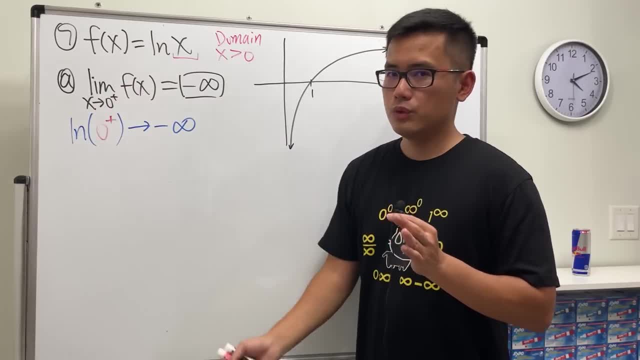 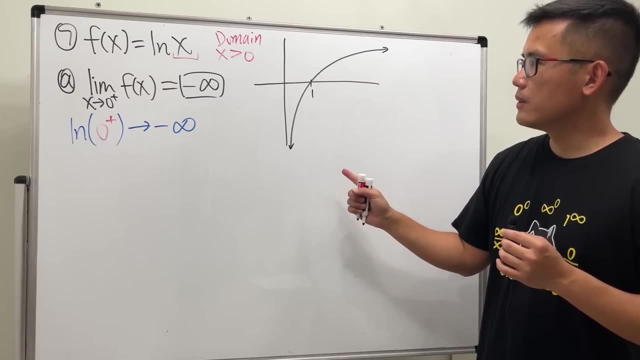 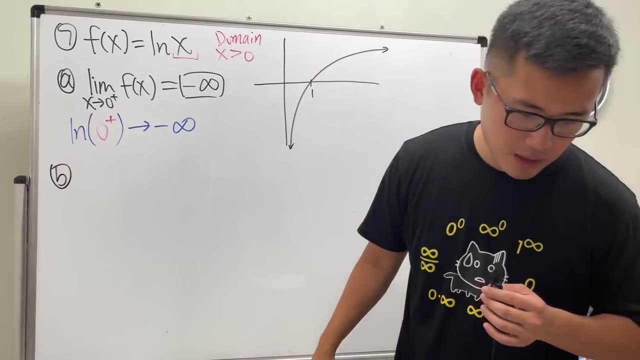 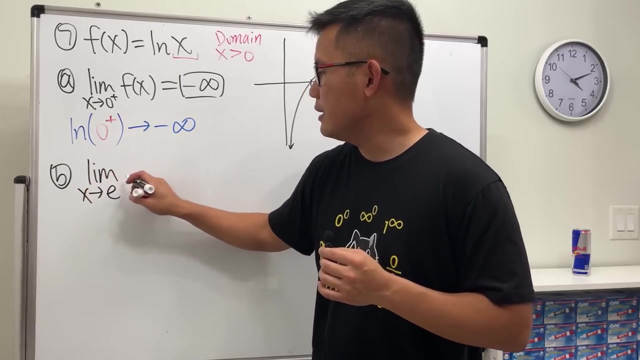 just zero wouldn't make sense. x approaching zero minus wouldn't make sense either. so so that. and then let me see what else do i want to mention. yeah, that's all. moving to the next one, b. okay, next one. limit as x approaching e of the function. 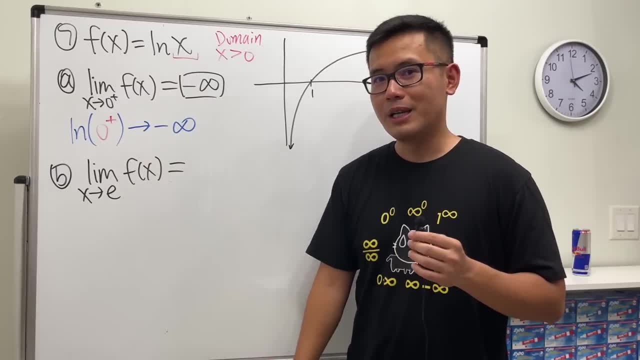 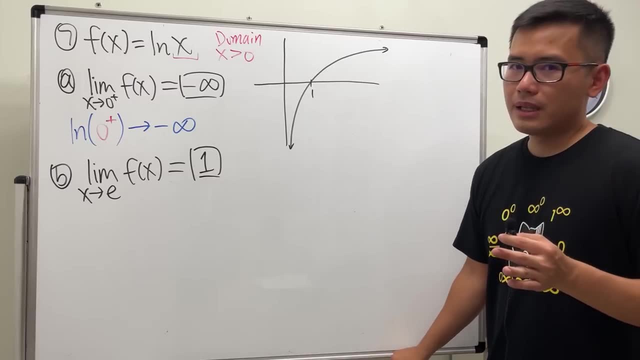 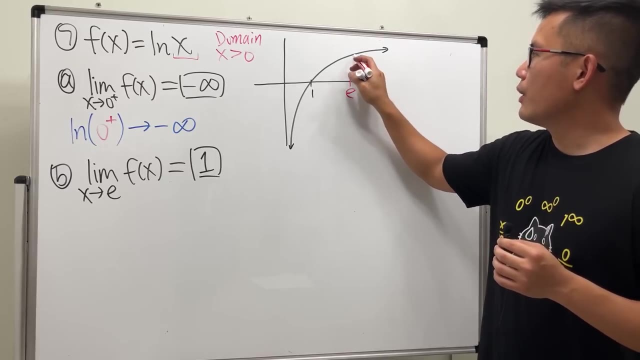 when x is approaching e, we can put e into ln x and guess what ln e is just equal to one. so the answer is just one. in fact, e is about like 2.718, right? so let's say e is about right here. when we put e into the ln function, you see how the function is nice and continuous. 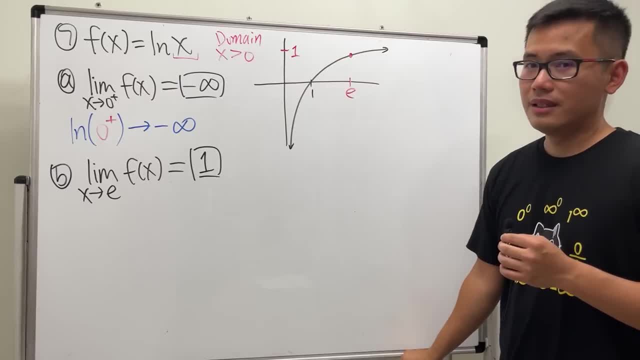 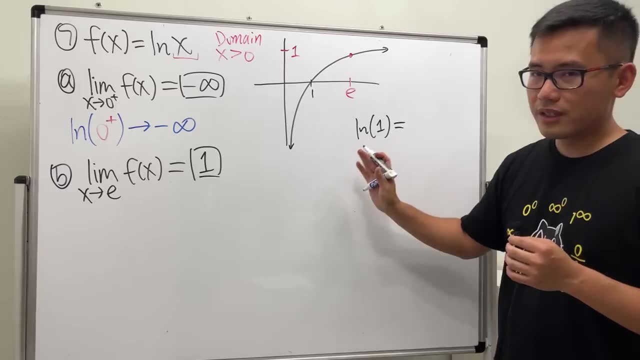 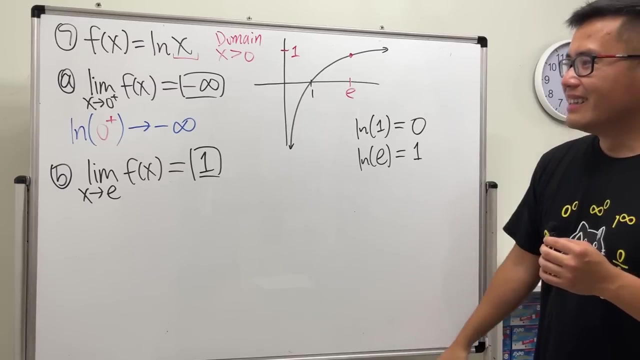 and the y value here is one. yeah, that's it. so some of the values that you definitely have to know: ln one- this is not limit, it's just a regular computation- and one is zero, and then ln e is one- okay, and then this right here is like the limit. so just remember that. 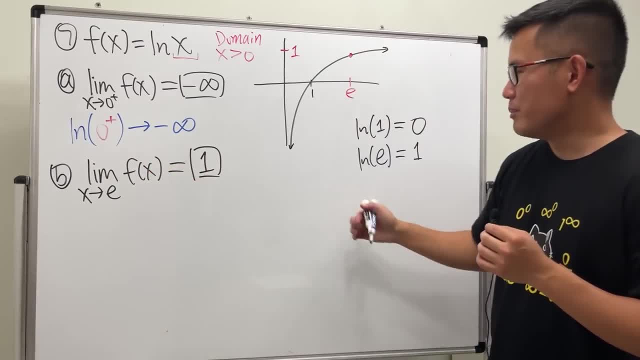 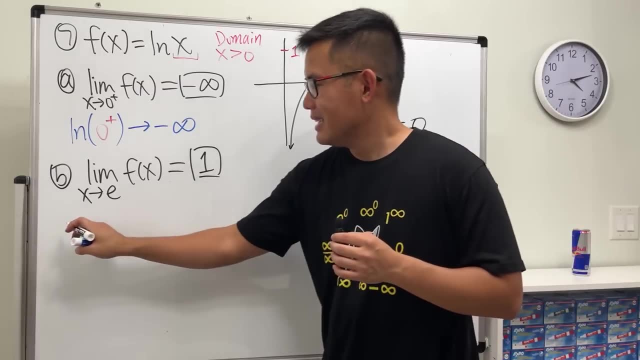 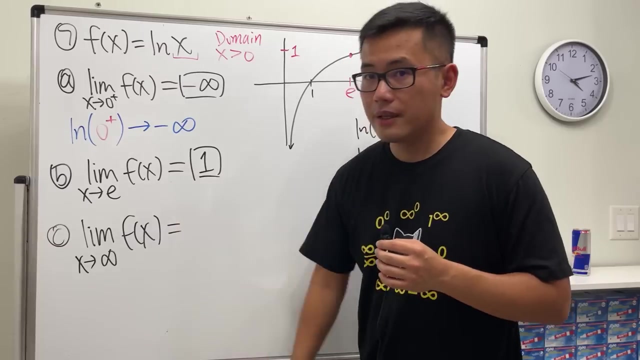 OK, And then this right here is like the limit. So just remember that if we have ln and then zero plus, this goes to negative infinity, And you know. the next one is the limit as X approaching infinity. You see how the curve is like this. 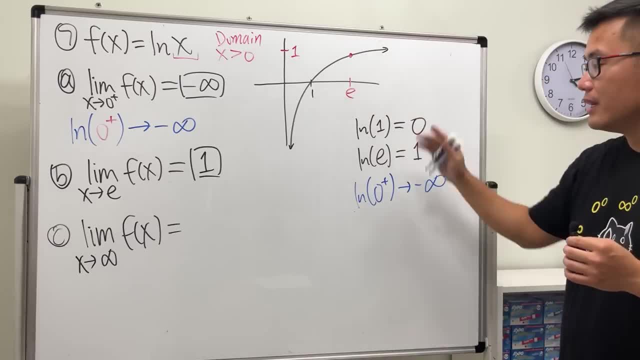 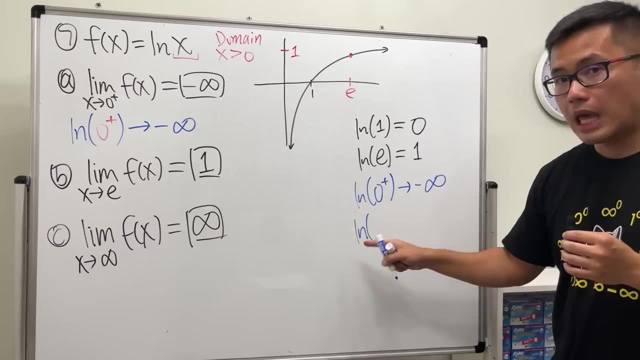 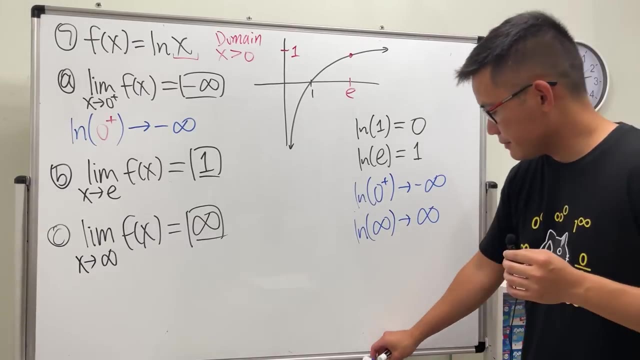 In fact, it's going to get bigger and bigger than the y-value. So this right here gives us infinity. So another expression that you should remember is ln. If you have infinity inside, E approaches positive infinity. So this is what we have. 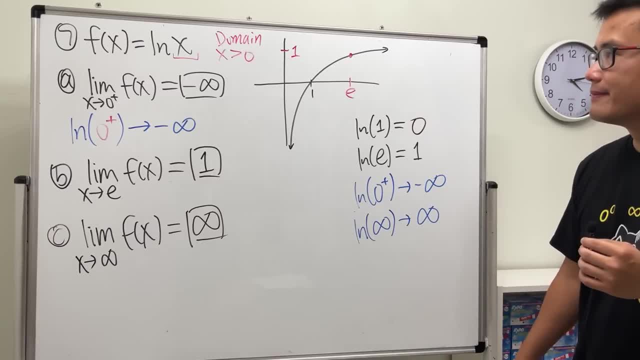 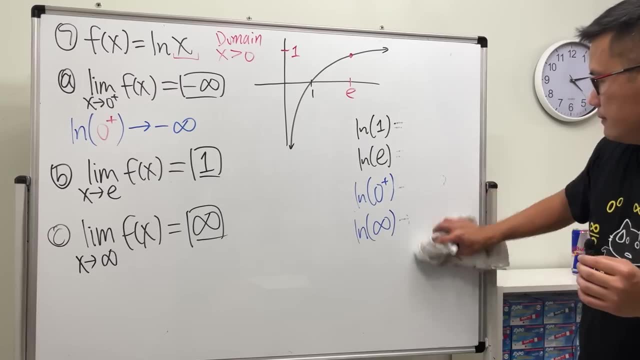 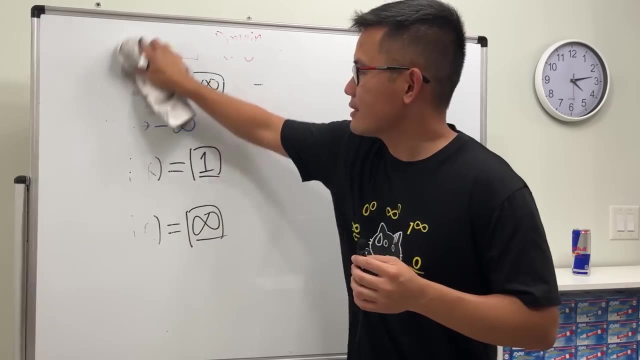 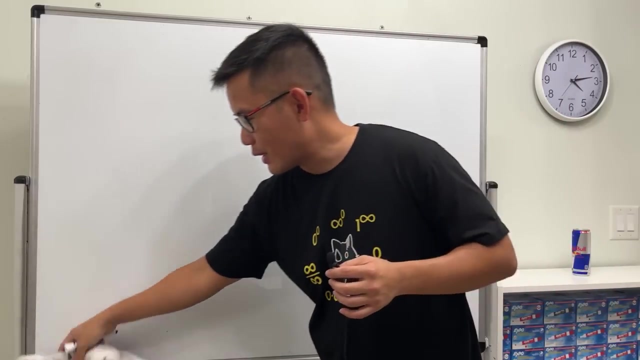 OK, so take a look. Take a look. OK. Well, number seven already. that's cool, And I think I'm just going to check to see if the phone is recording every 10 questions, So that way I can have a peace of mind. 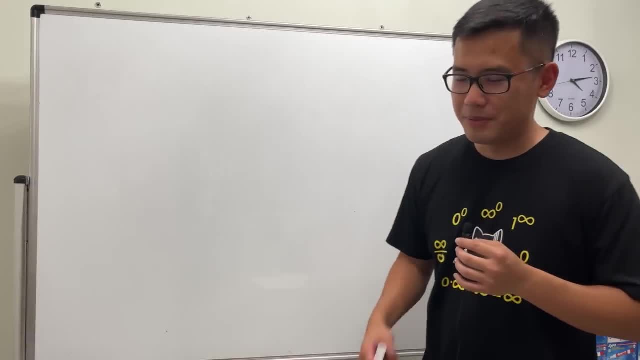 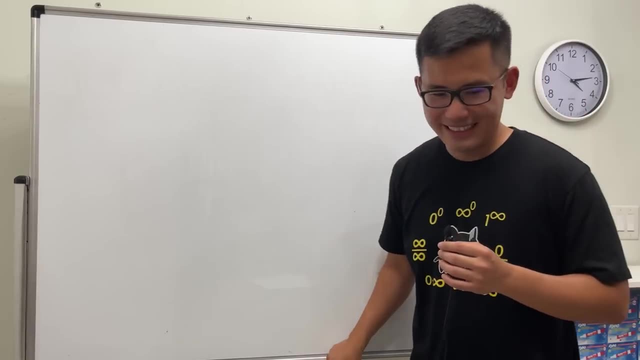 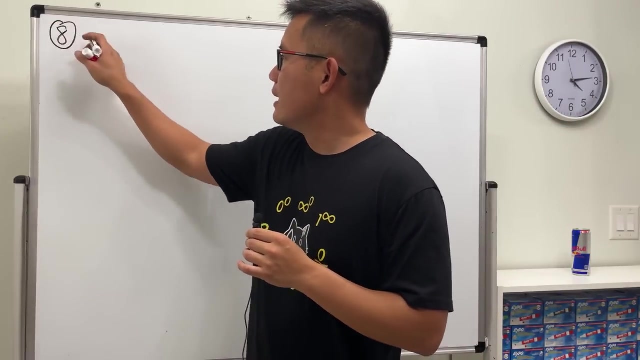 And, to be very honest with you guys, I do not have a peace of mind because I dropped the microphone earlier. Hopefully the sound is OK. If it doesn't, I will record it again, Don't worry. Anyway, number eight: Aha, our function earlier was ln X. 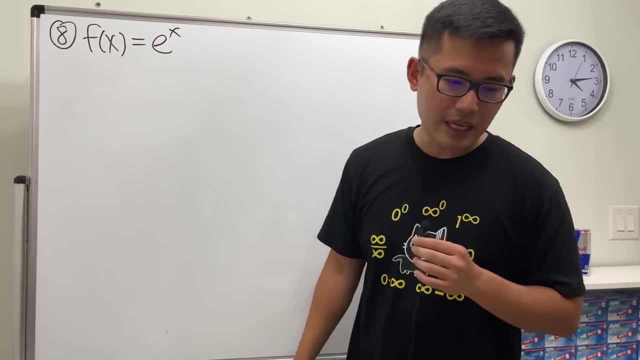 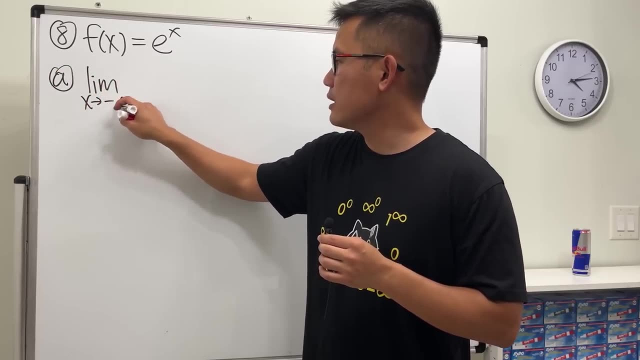 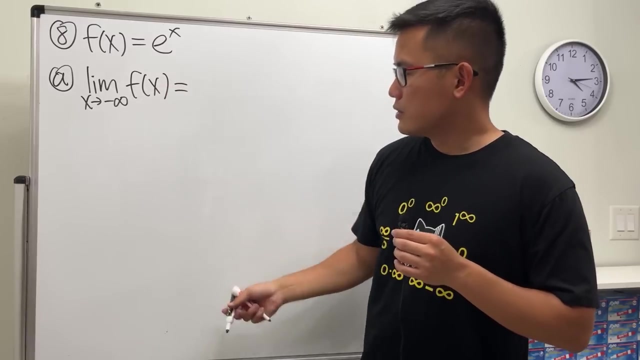 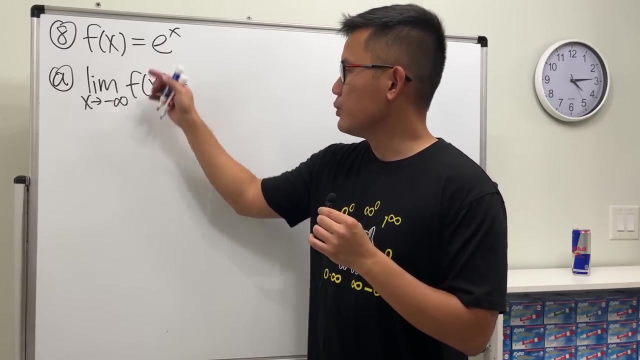 You expected, here we have E to the X. OK, So part A. let's look at the limit as X approaching negative infinity of the function. So again, if you don't use graph, maybe just want to like plug in and kind of reason out. this is how you can do it: Put negative infinity to here. 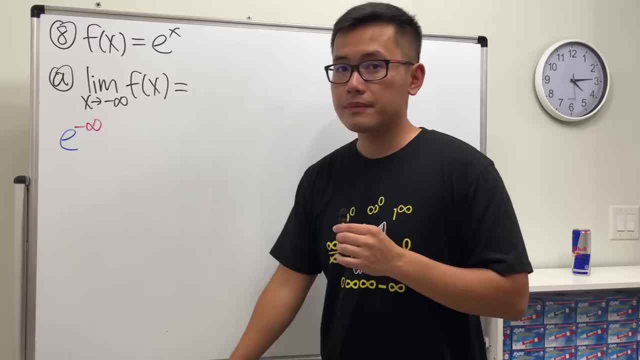 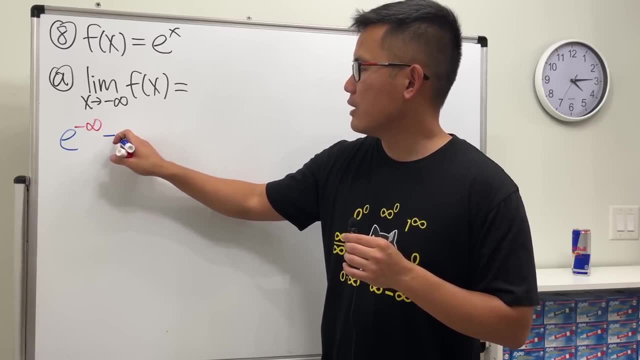 So we are looking at E to the negative infinity And you see we have negative exponents. So maybe, if you want to, you can just say this: right, here is a technical: yeah, we'll put equal, because it's like computation in the negative. 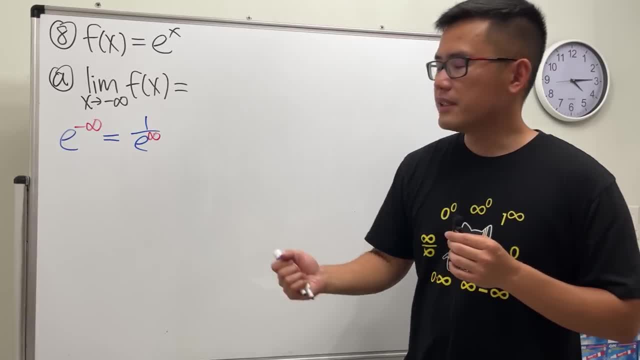 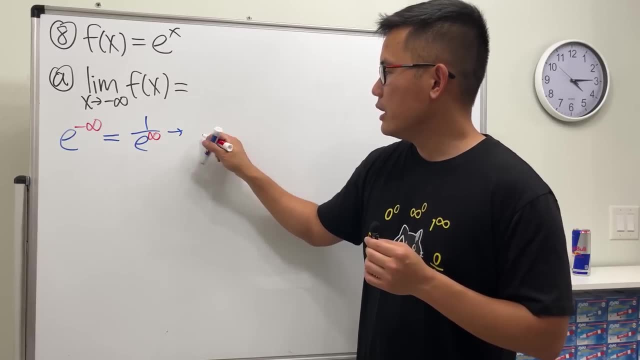 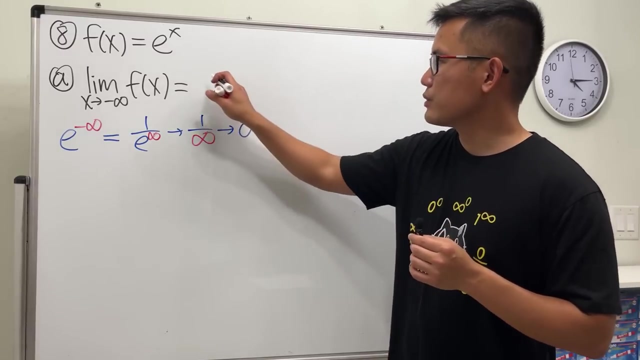 So it's 1 over E to the infinity. And here's the deal: E is 2.718. each Raised to infinity's power equals to infinity, And 1 over infinity is approaching zero, All right. So this right here is zero. 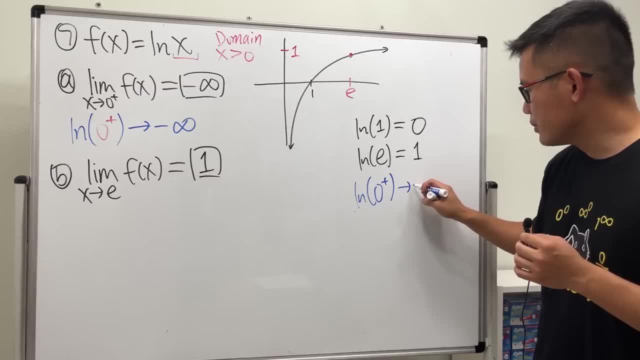 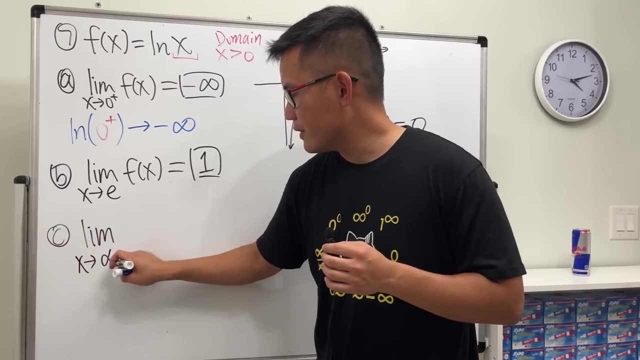 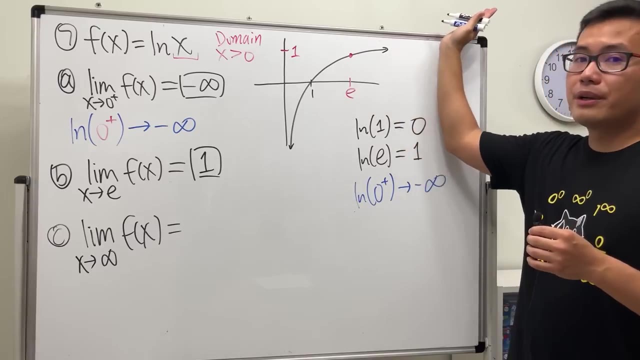 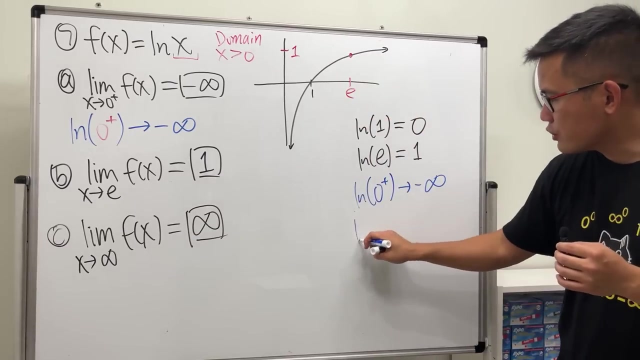 if we have ln and then zero plus, this goes to negative infinity, and you know the next one is the limit as x approaching infinity. you see how the curve is like this. in fact, it's going to get bigger and bigger, like the y value. so this right here gives us infinity. so another expression that you should remember is: 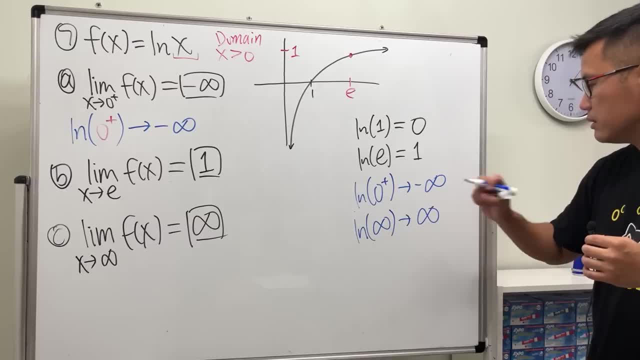 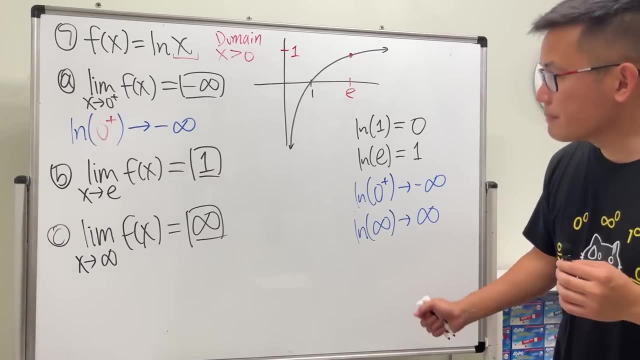 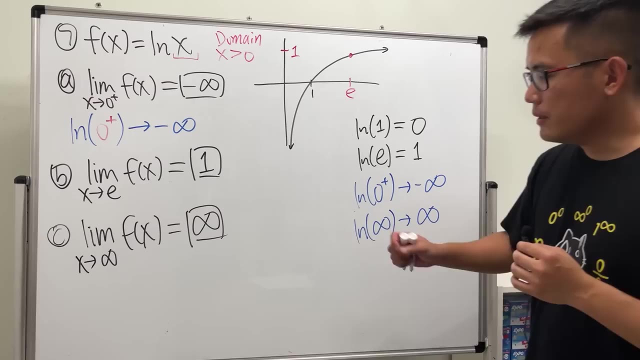 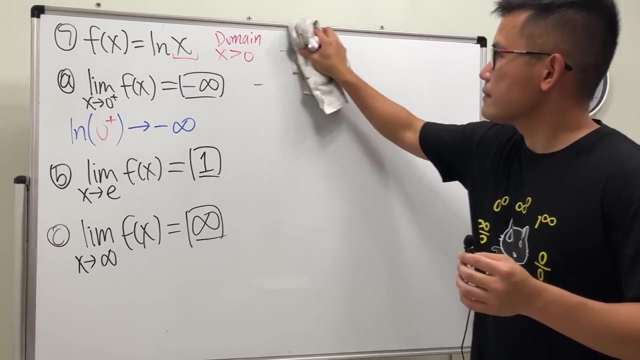 ln. if you have infinity inside, it approaches positive infinity. so this is what we have, okay, so take a look, take a look, okay, wow, number seven already. yeah, that's, that's cool. okay, so this is what we have. so now you see that already, if y approaches positive infinity, 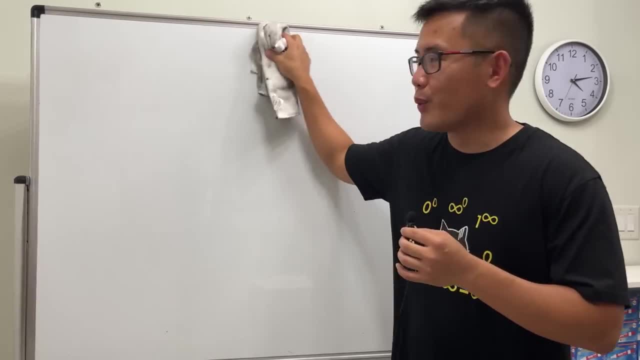 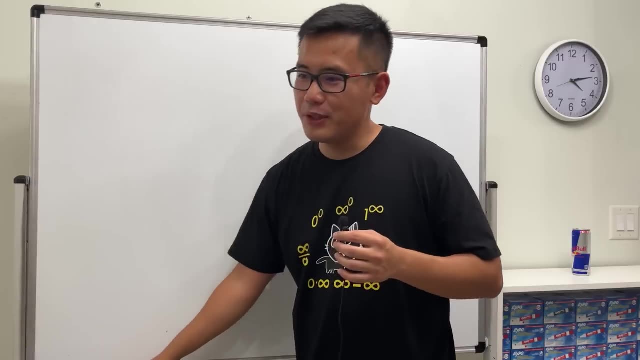 and i think i'm just going to check to see if, if the phone is recording every 10 questions so that way i can have a peace of mind. and, to be very honest with you guys, i do not have a piece of mind because i dropped the microphone earlier. hopefully the sound is okay, if it doesn't. 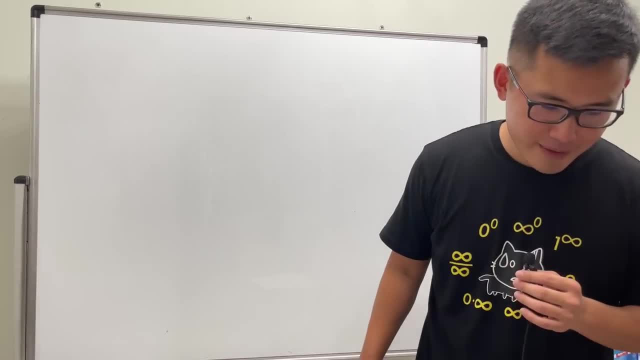 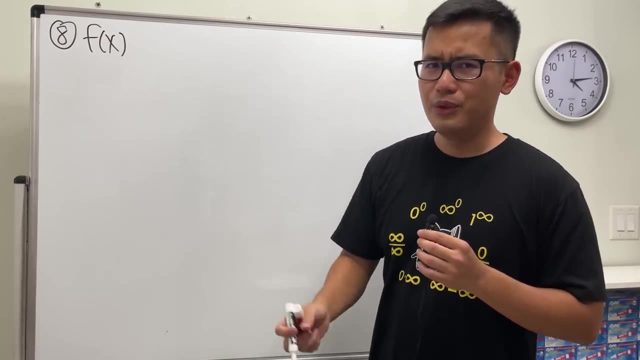 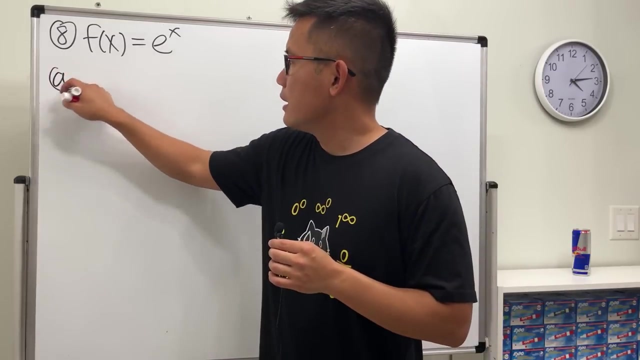 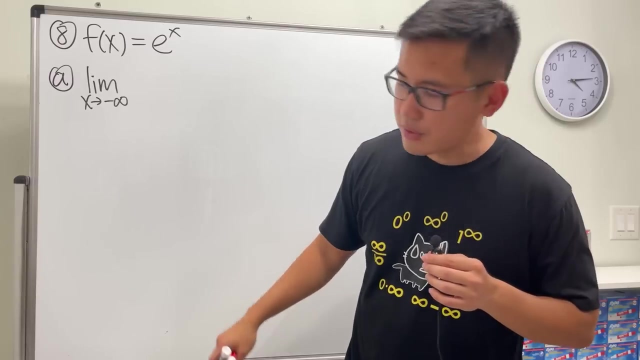 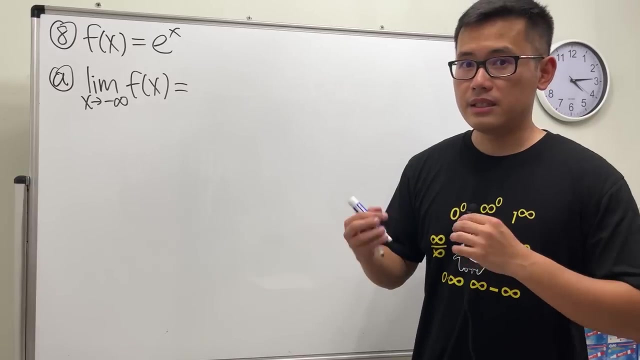 i will record it again, don't worry. um, anyway, number eight: aha, our function. earlier you was lnx, you expected. here we have e to the x. okay, so part a. let's look at the limit as x approaching negative infinity of the function. so again, if you don't want to use graph, maybe just want to like plug in and kind. 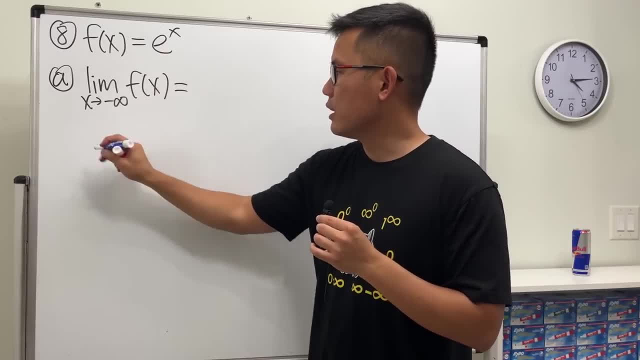 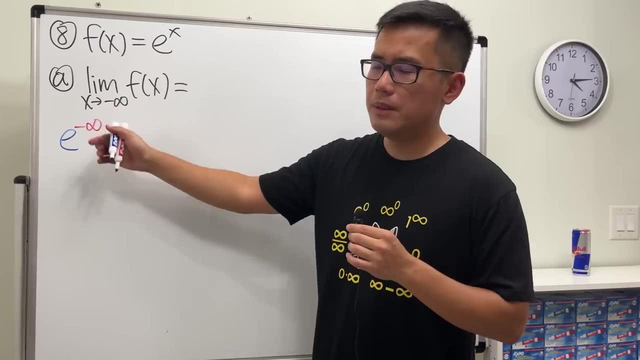 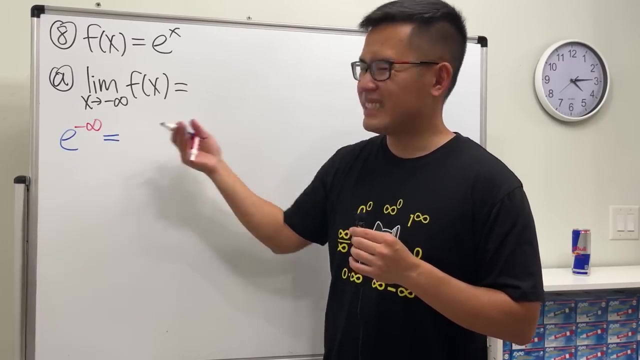 of recently out. this is how you can do it: put negative infinity to here. so we are looking at e to the negative infinity and you see we have negative exponents. so maybe, if you want to, you can just say this right: here is: uh, technically i will put equal, because it's like computation. 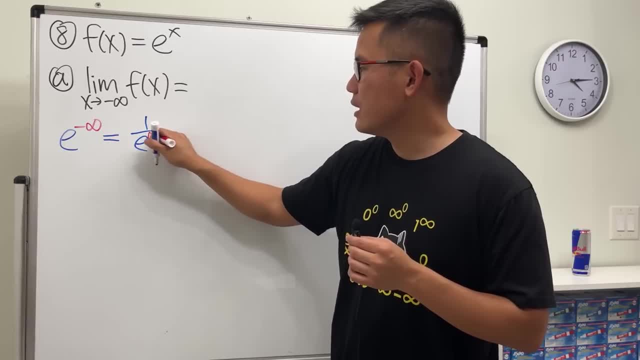 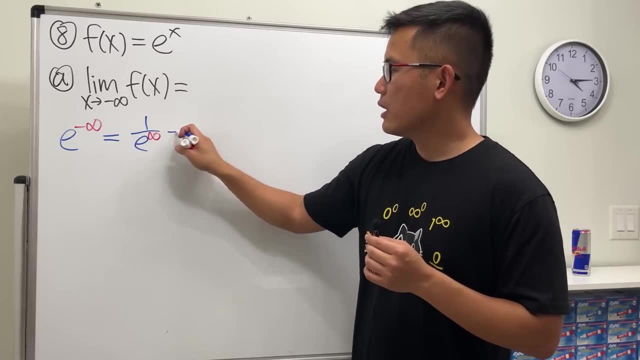 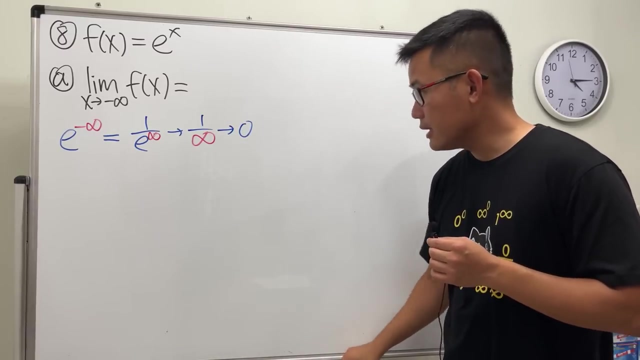 in the negative right. so it's one over e to the infinity. and here's the deal: e is 2.718, yeah, each raised to infinity's power, it goes to infinity, and one over infinity is approaching zero. all right, so this right here is zero, okay. 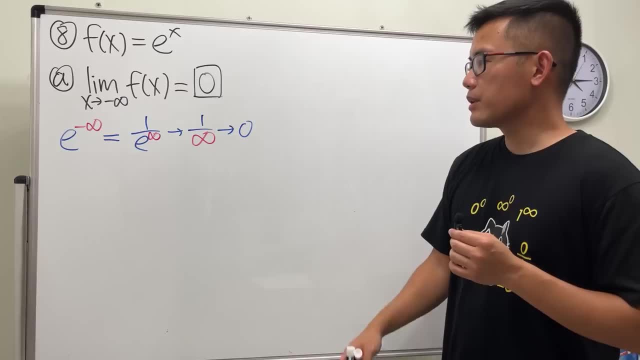 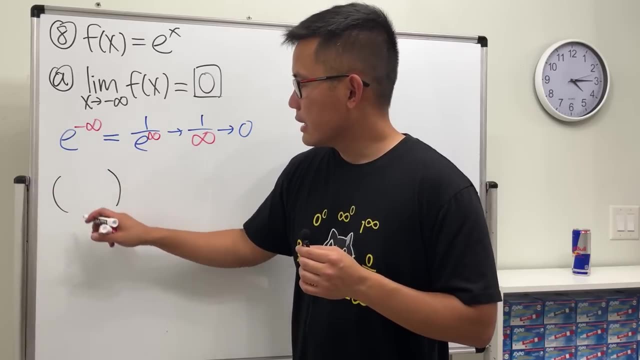 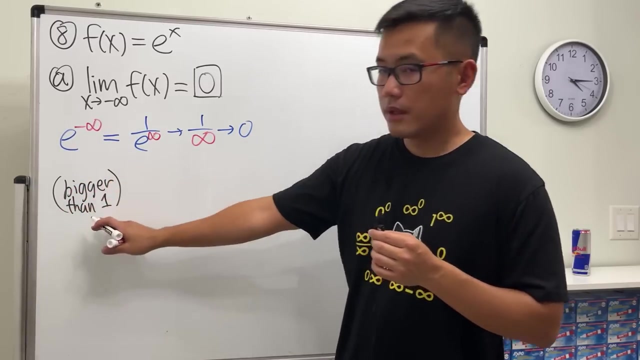 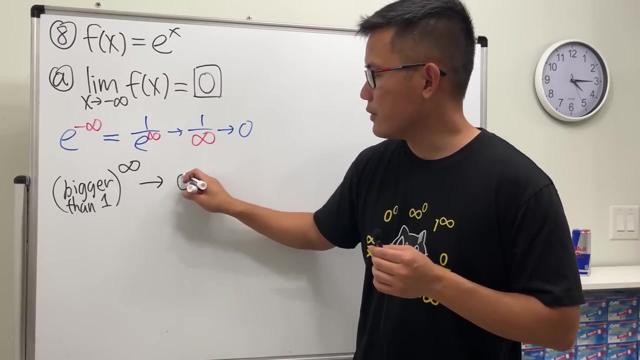 OK, so this right here, perhaps I'll tell you guys this thing Real quick. The deal is that if we have a base, if we have a base that's bigger than one, Bigger than one, If we have this raised to the infinity's power, this right here will go to infinity. 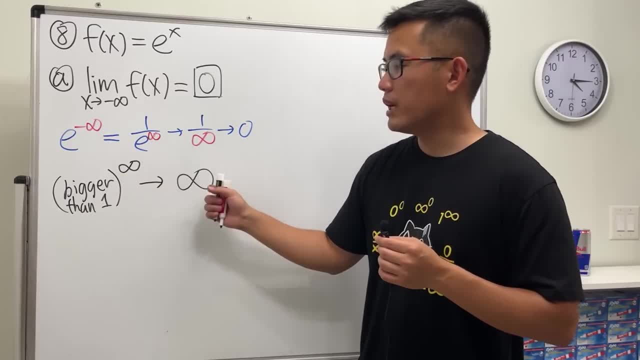 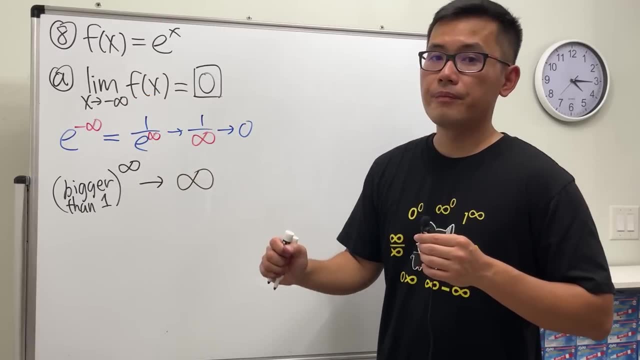 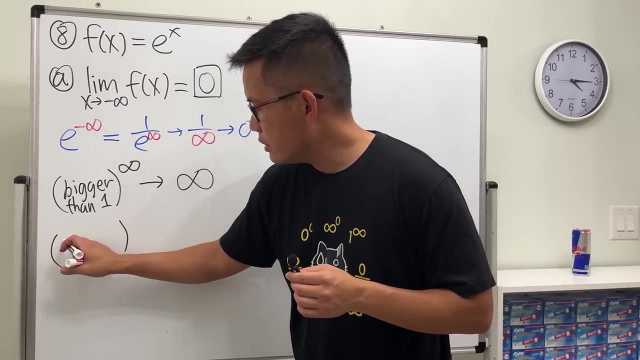 Let's say 1.001 raised to infinity's power, we get infinity. All right, E is 2.7 each, So that's why The bottom it goes to infinity. Another way to look at this is that if we have a base, that's in between. 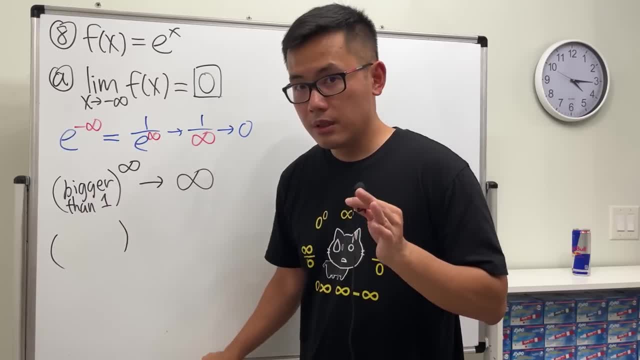 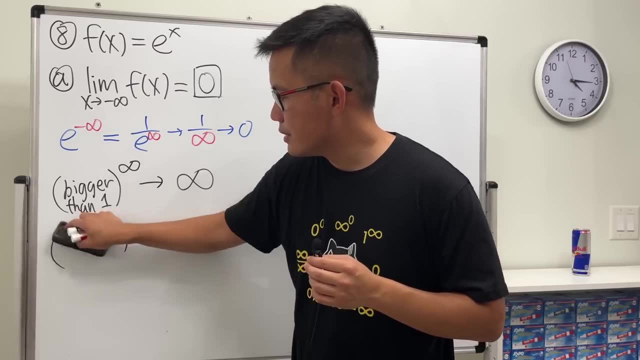 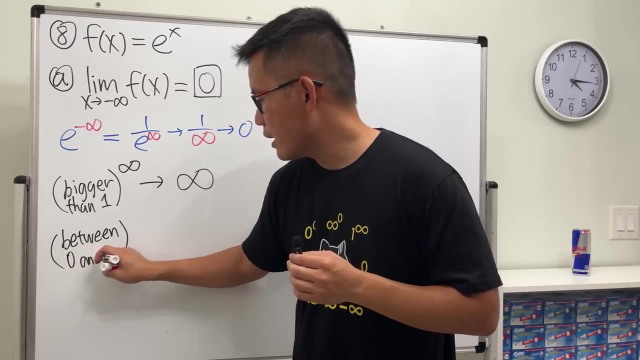 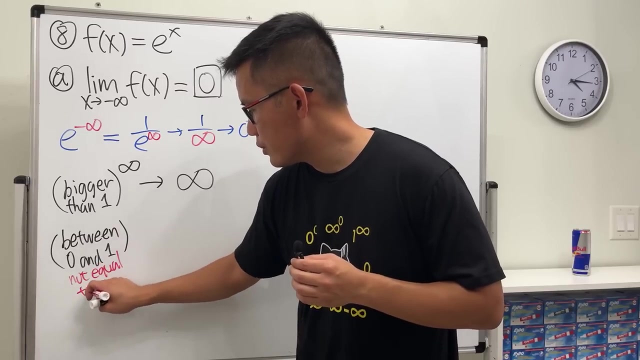 between- I will say this- between zero and one. So I will just say: Hmm, I'll say this: between- Let's use the word between- between zero and one, but not equal to one, not equal to one, And then raised to the infinity's power. 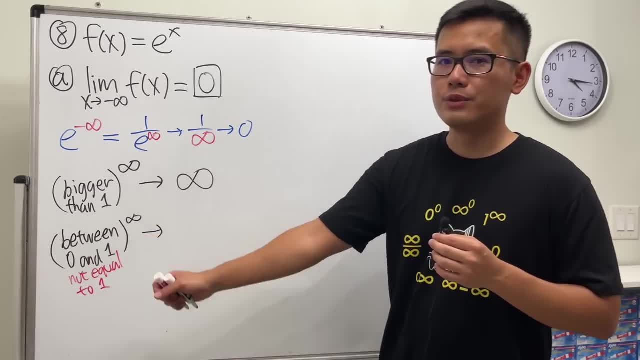 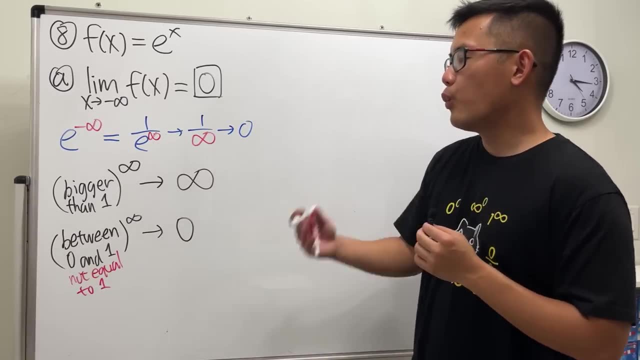 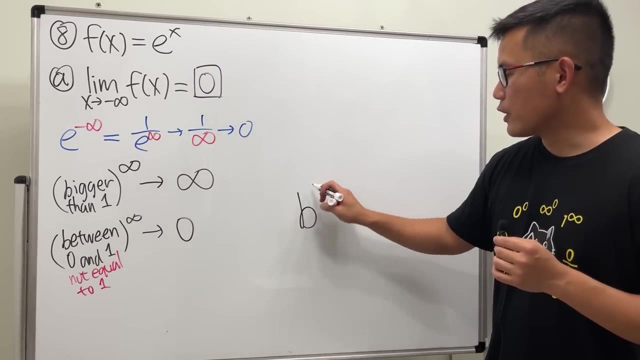 Now say one half or zero, or 0.001.. Raised to infinity's power, we can say that this is approaching zero. And you might be wondering what if we have a base that's less than zero? Well, if you're talking about functions, when we have a function written in this form, b to the x power, 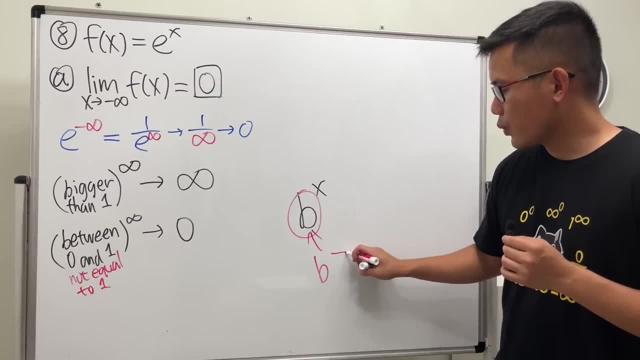 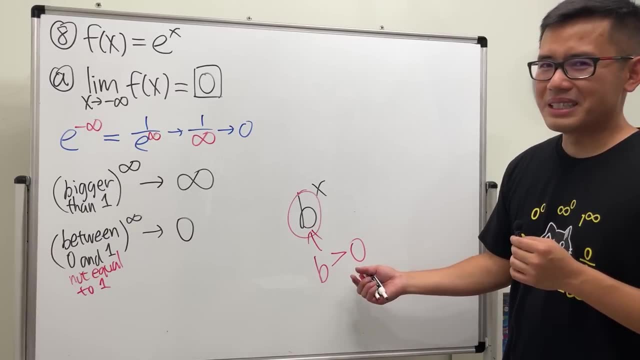 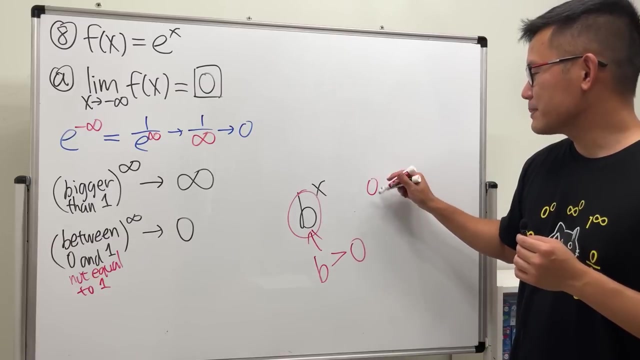 we will have to make sure that the base b is greater than zero. Yeah, Technically you can say b greater than or equal to zero, but like zero to the x power, it's almost always zero, right? But yeah, anyway, zero to the x power. this right here. x cannot be negative numbers. 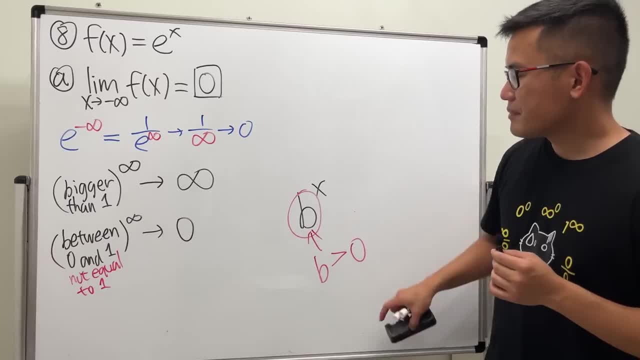 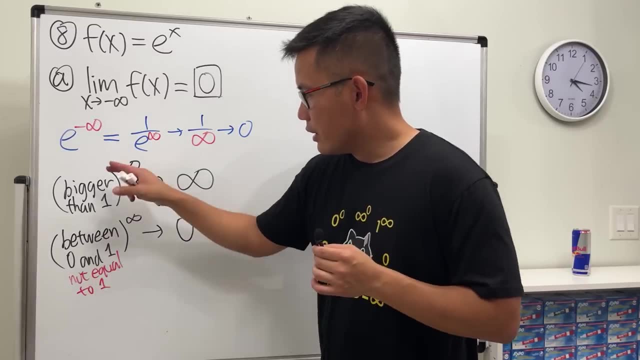 Otherwise we divide it by zero. But yeah, when we have exponential function, b wants to be greater than zero. That's why, Okay, So again, when the base is bigger than one, to the infinity's power is infinity, we can draw a conclusion. 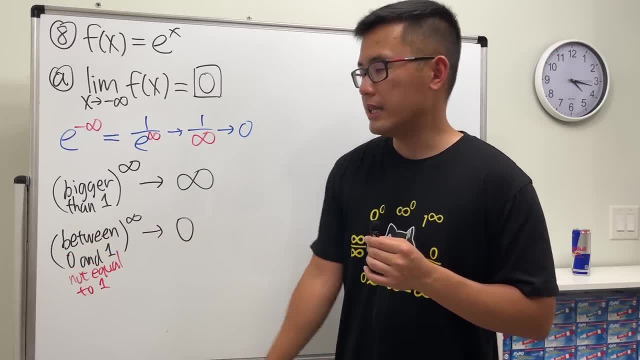 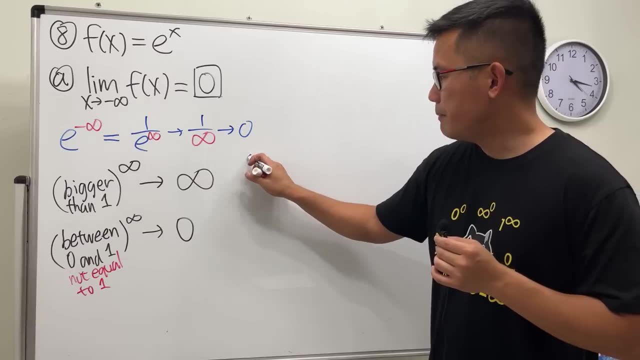 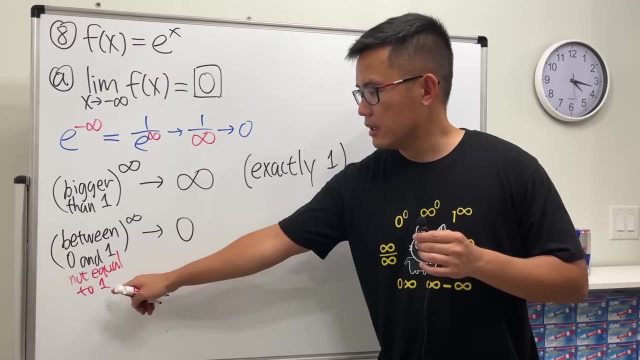 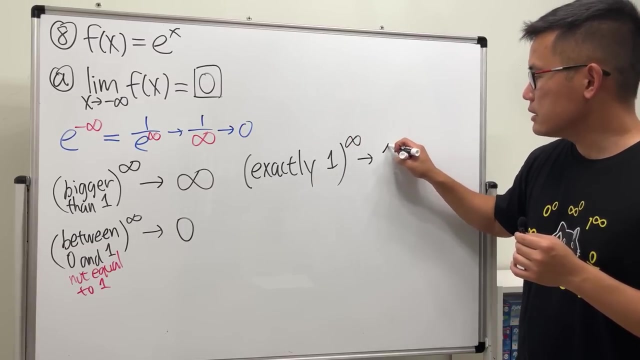 If it's between zero and one, not equal to one, then we get zero. Okay. And then I also want to mention: if the base is exactly equal to one- Just like earlier I said, not exactly, not equal to one- If it's exactly equal to one and then raised to infinity's power. this right here is: 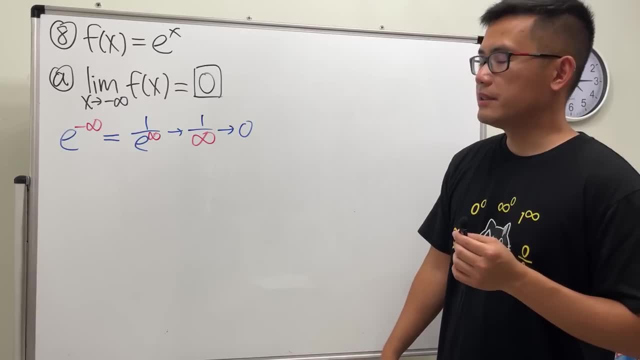 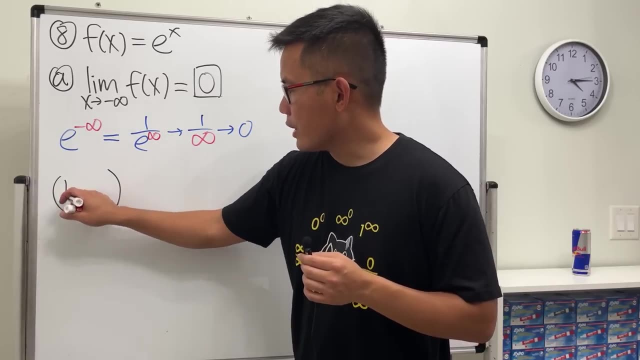 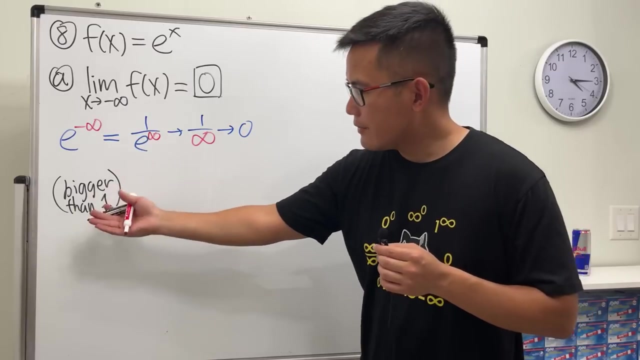 so this right here, um, perhaps i'll tell you guys this thing real quick. the deal is that if we have a base right, if we have a base that's, uh, bigger than one, bigger than one, if we have this raised to the infinity's power, this right here will go to infinity. 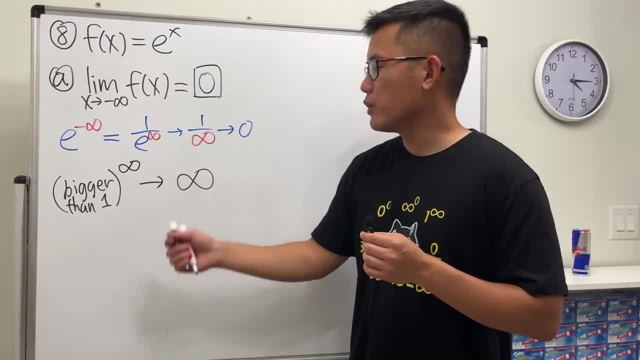 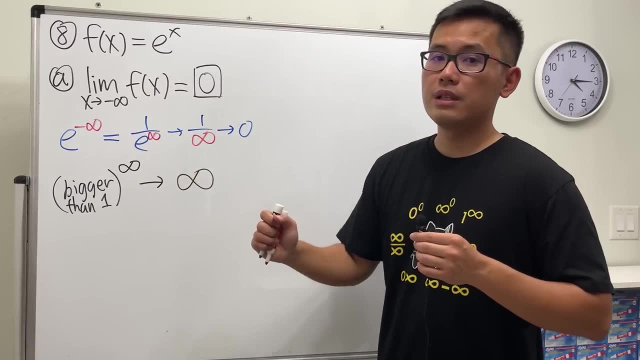 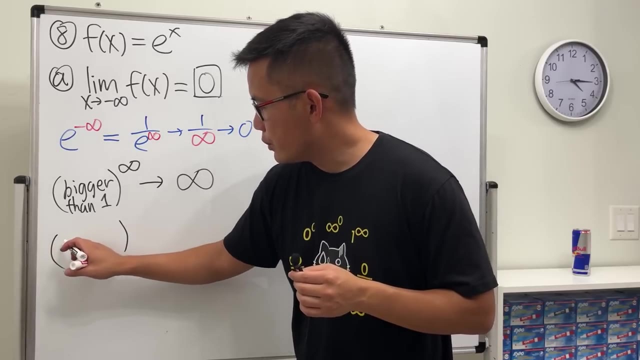 let's say 1.001 raised to infinity's power, we get infinity. all right, e is two point seven entropy. so that's why, if you look at the bottom, it goes to infinity. um, another way to look at this is if we have a base that's in between between, i would say, if we are looking at the. 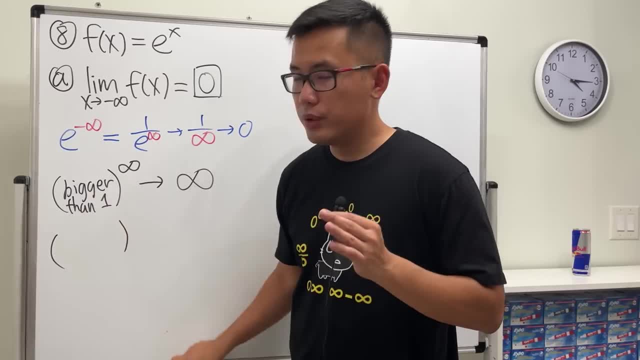 third line. i will say this because during an FMQ million, what i'm going to give you guys is to take that 0 push and you are going to duplicate this right here. so I've got e to the right, so i will say so far, e to theต. raise to infinity. so when you raise to infinity's power, you 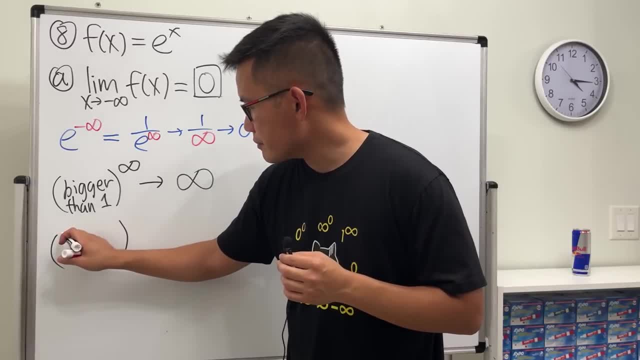 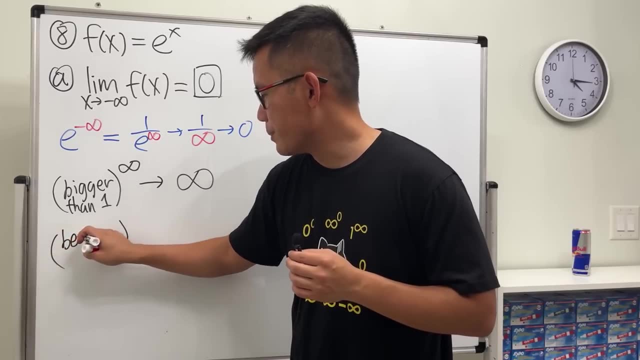 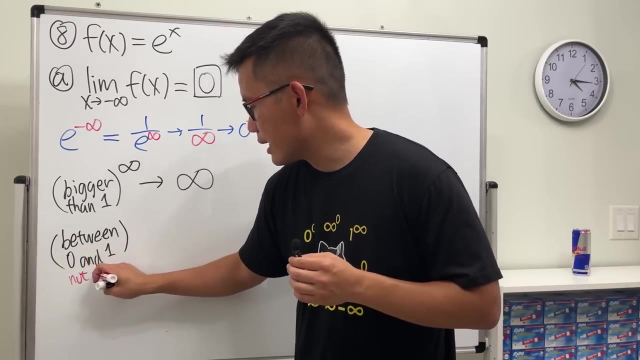 get to infinity, all right, e is 2.78. so that's why, if you look at the bottom, it goes to infinity another way: to94. também. So I will just say, I'll say this: between- yeah, let's use the word between- between 0 and 1,, but not equal to 1,, not equal to 1.. 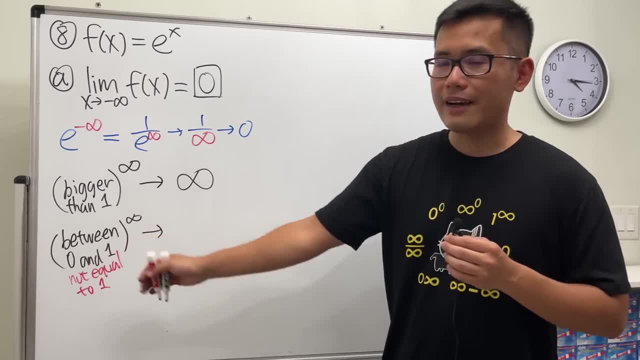 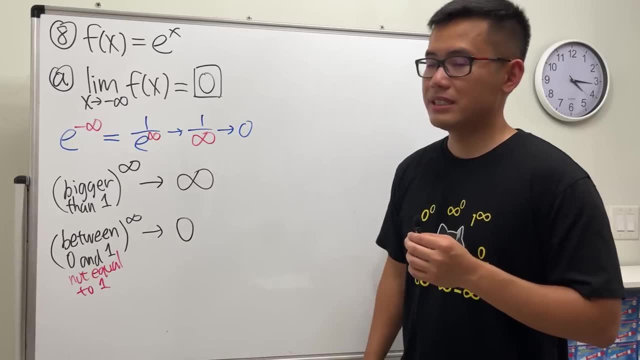 And then raise to the infinity's power. Now say 1 half or 0 or 0.001.. Now raise to infinity's power. we can say that this is approaching 0.. And you might be wondering what if we have a base that's less than 0?? 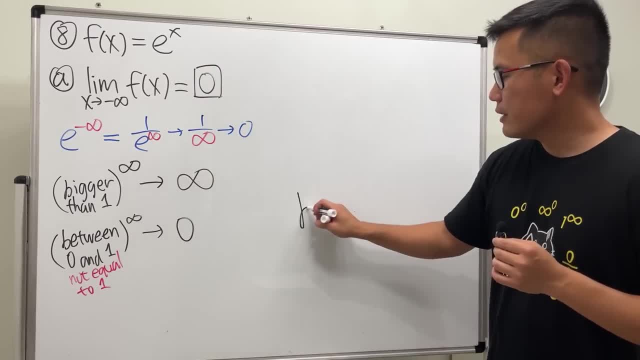 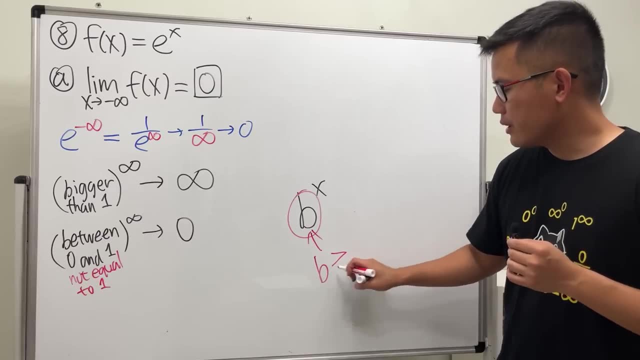 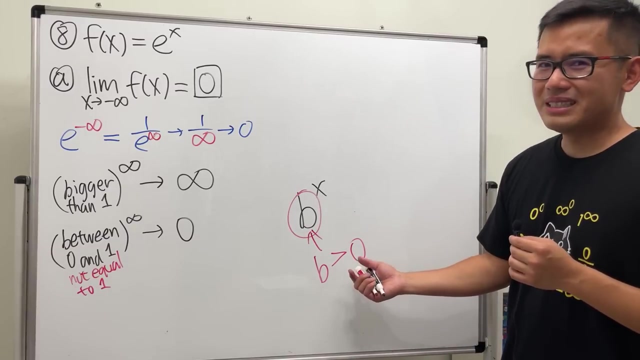 Well, if you're talking about functions, when we have a function written in this form, b to the x power, we will have to make sure that the base b is greater than 0. Technically you can say b greater than or equal to 0, but like 0 to the x power. 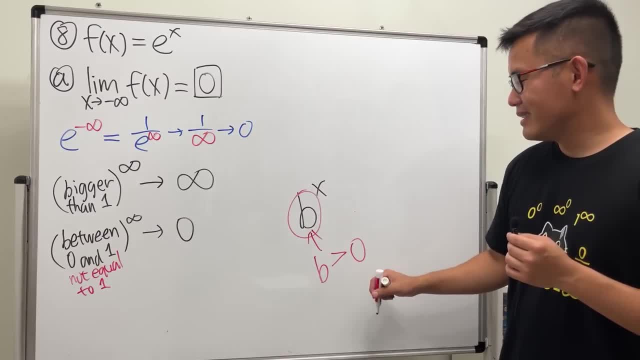 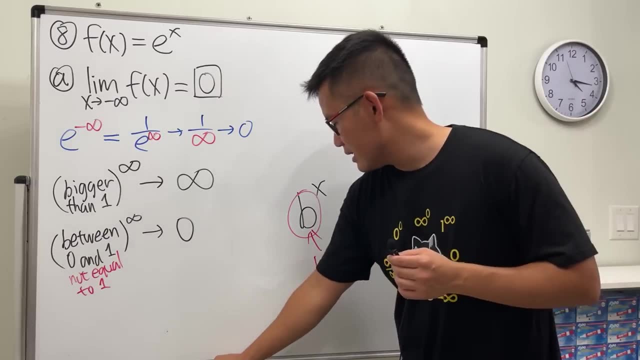 it's almost always 0,, right, But yeah, anyway, 0 to the x power. this right here. x cannot be negative numbers, otherwise we divide it by 0, but yeah, when we have an exponential function. 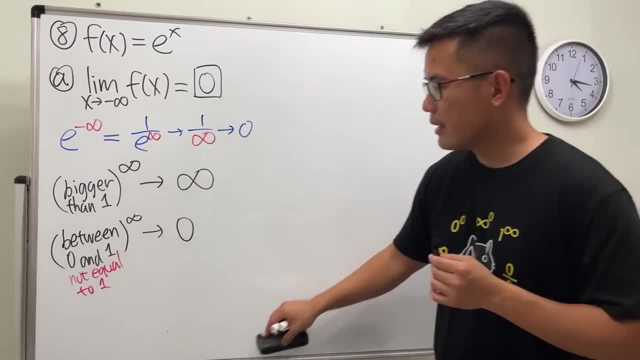 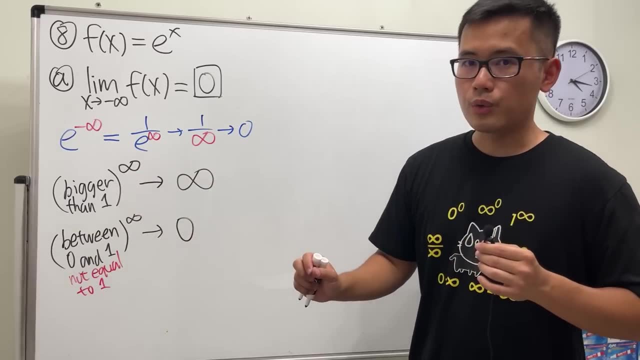 b wants to be greater than 0,. that's why okay. So again, when the base is bigger than 1, to the infinity's power, it is infinity. we can draw a conclusion: If it's between 0 and 1, not equal to 1, then we get. 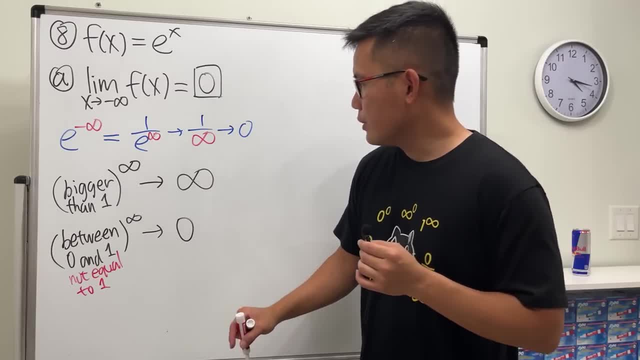 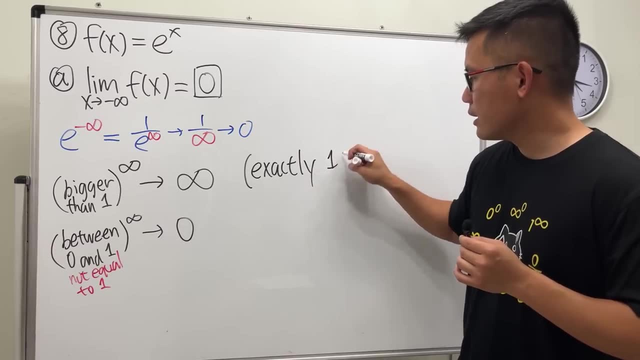 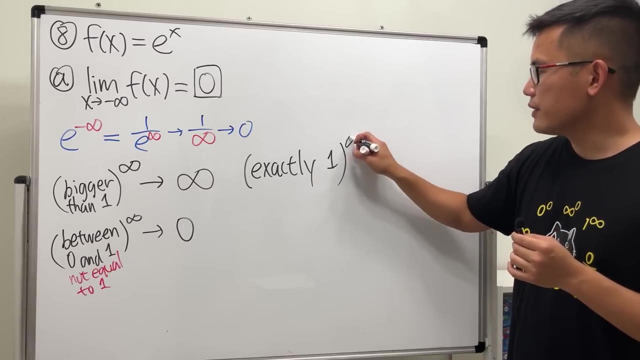 0, okay. And then I also want to mention if the base is exactly equal to 1, just like earlier I said, not exactly, not equal to 1, yeah, If it's exactly equal to 1 and then raised to infinity's power. 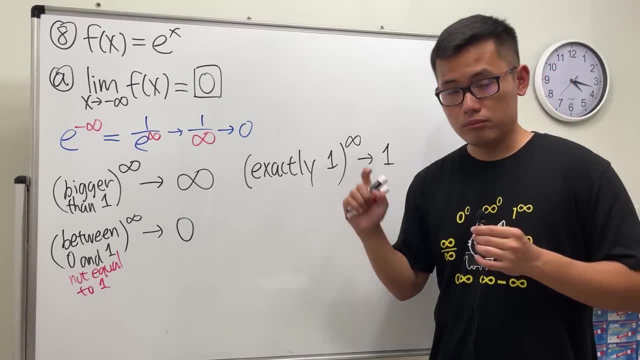 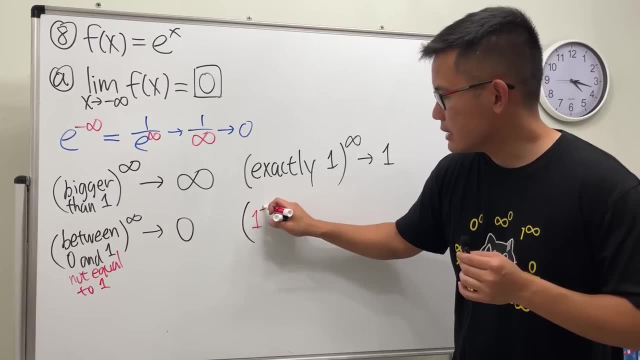 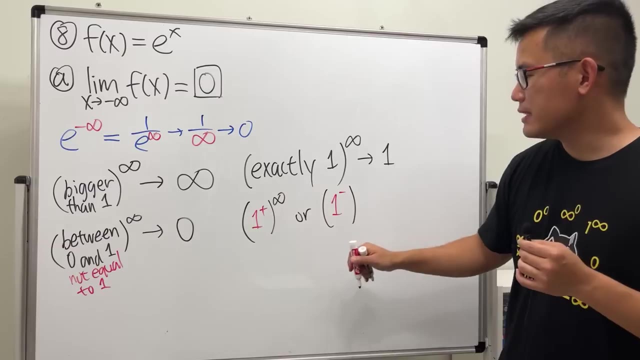 this right here is approaching 1, okay. However, if you get, let's say, 1 plus 2, to the 0's power, or 1 minus, sorry, 1 plus 2 to infinity's power, or 1 minus to the infinity's power, one or the other, 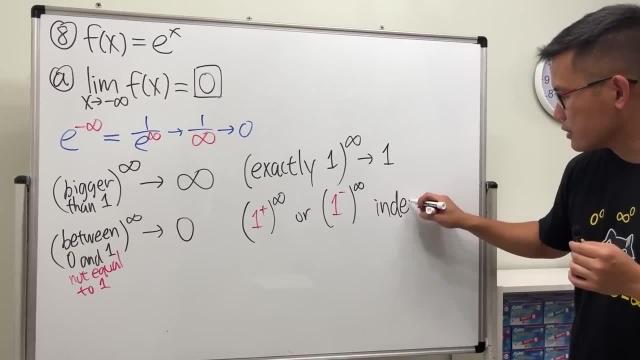 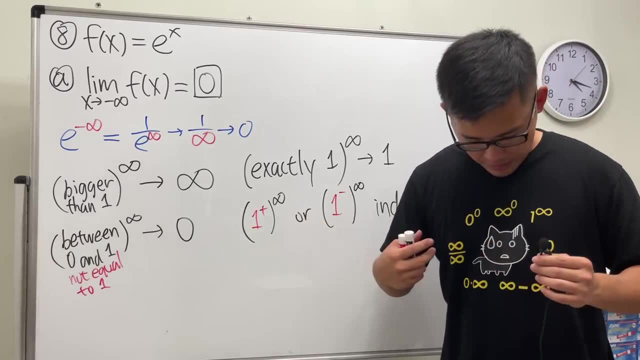 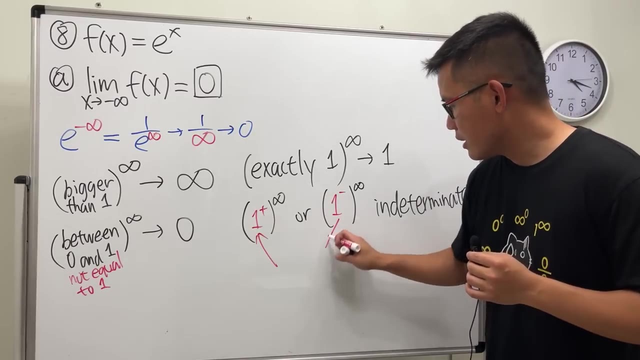 this right here, right this, right here. they are the so-called indeterminate form, meaning that we do not know what the answers are. Why? Well, it's not much. sure you know what I mean? No, Now, jokes aside. here, this right here, are the limit form. 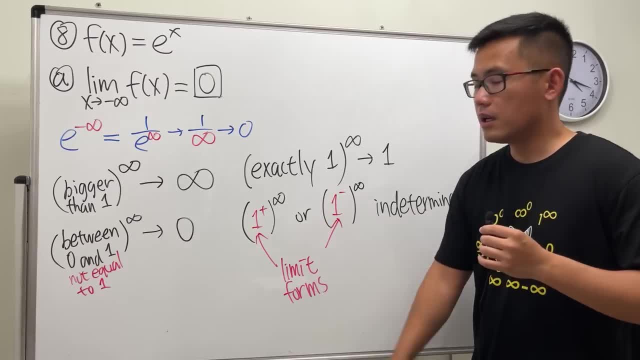 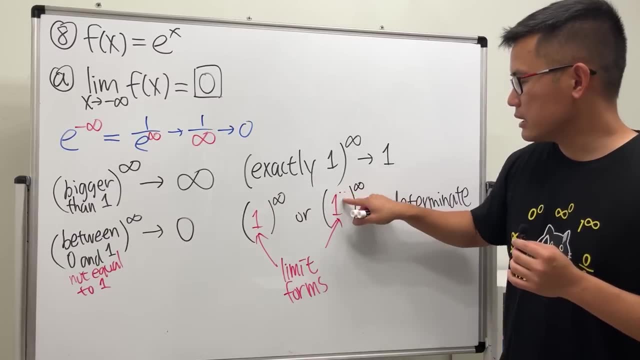 and the crazy part- or like the dangerous part- of this is that a lot of times we don't even put a plus or minus. That's why you see my shirt right here we have a 1 to the infinity's power. 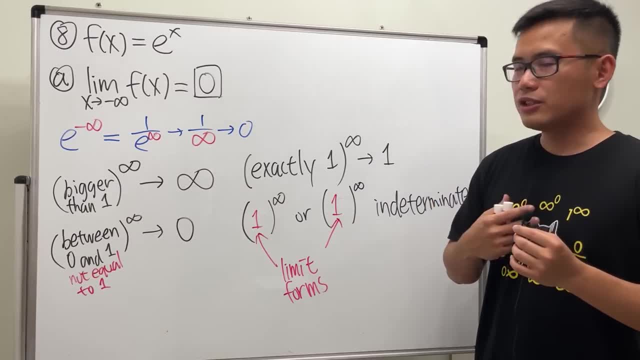 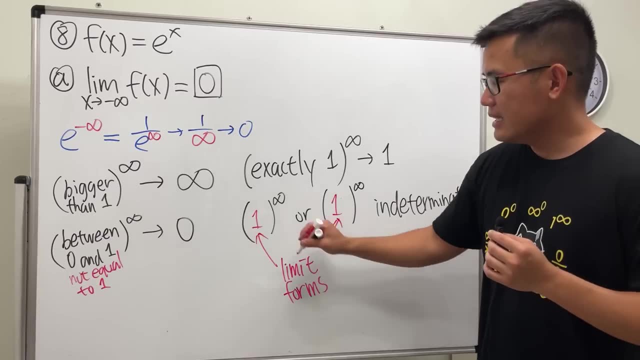 A lot of times it's misunderstood that, hey, it shouldn't not just be equal to 1.. No, No, This right here, this 1, it's a limit form, meaning that it's technically saying 1 plus or 1 minus. 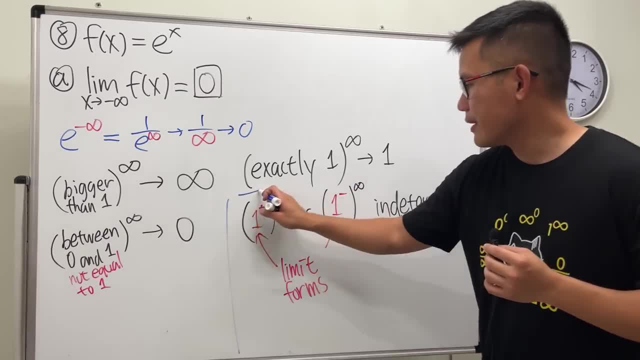 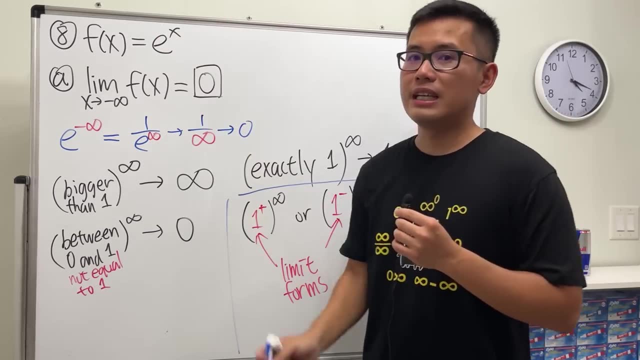 So this, right here, it's one of the most confusing part, and I would like to just give you guys an example before we go, especially when we're talking about e- to the x power, right. So the famous example for this one is: 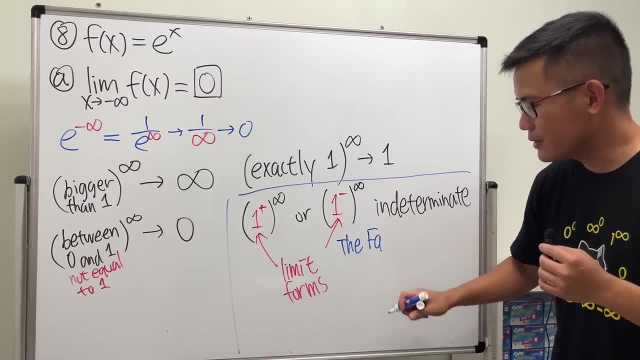 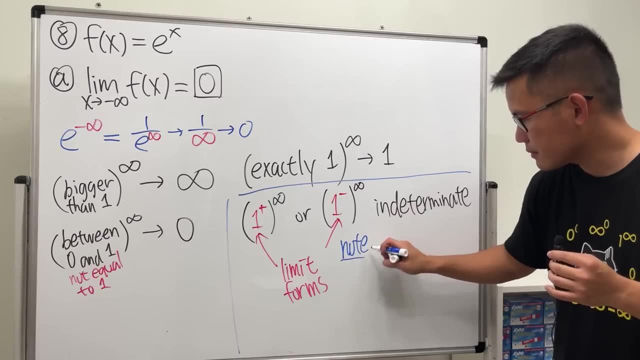 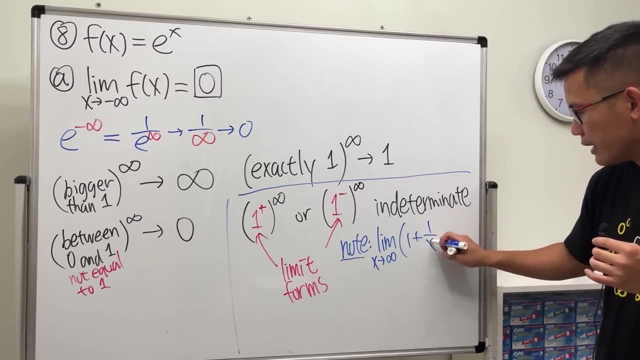 this is called the fact. Well, actually no, I'm not going to tell you guys the secret weapon yet. I'm just going to put down a note. If we have the limit as x approaches, say infinity, 1 plus 1 over x to the x power. 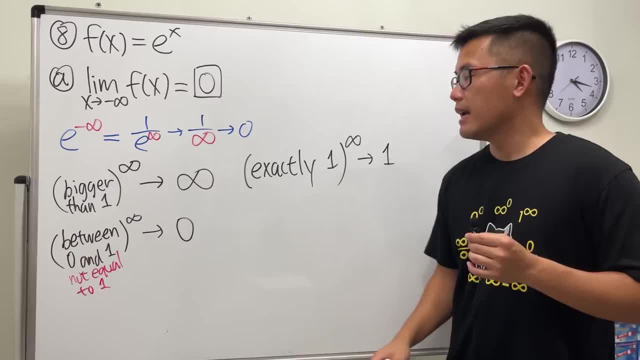 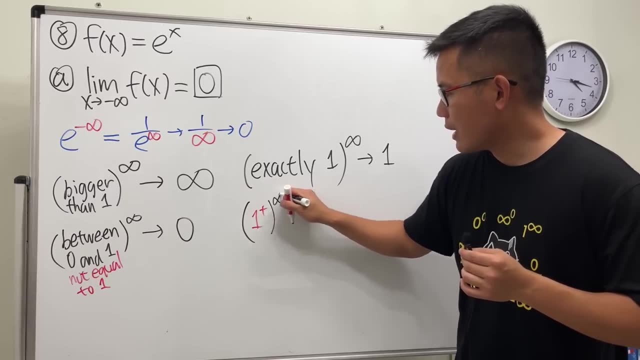 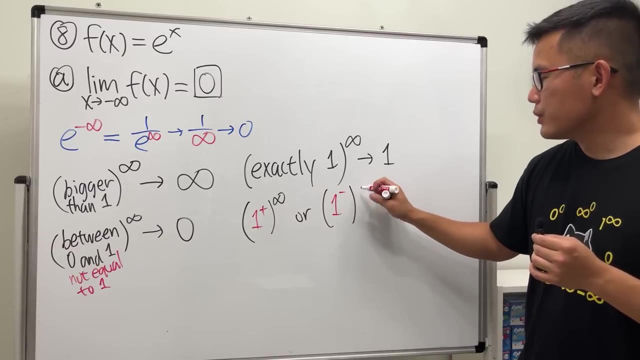 approaching one, Okay. However, if you get, let's say, one plus to the zero's power or one minus, sorry, one plus to infinity's power or one minus to the infinity's power, one or the other, this right here, right, this right here. 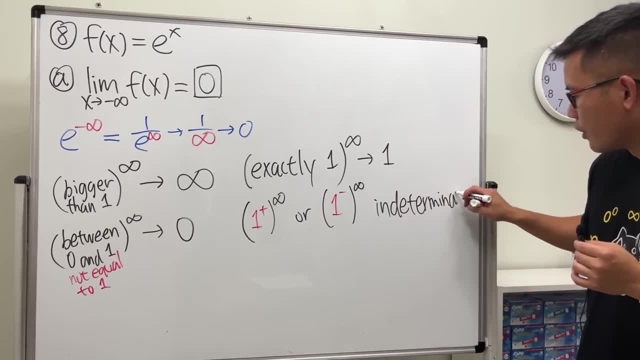 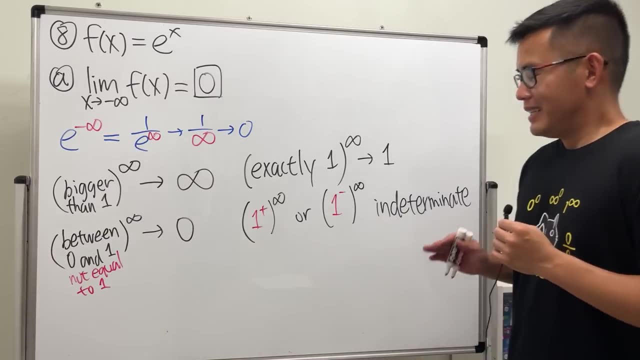 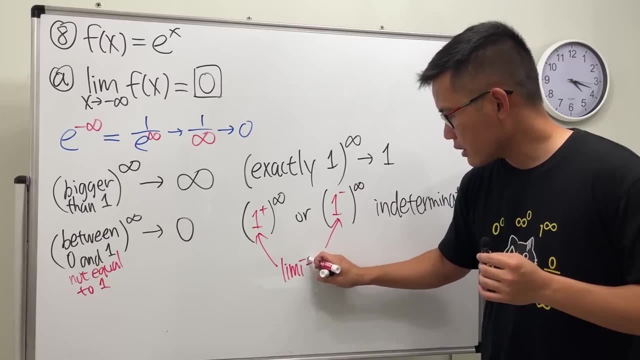 they are the so-called indeterminate form, meaning that we do not know what the answers are. Why It's on my shirt already. No Jokes aside here. this right here are the limit form And the crazy part, or the dangerous part. 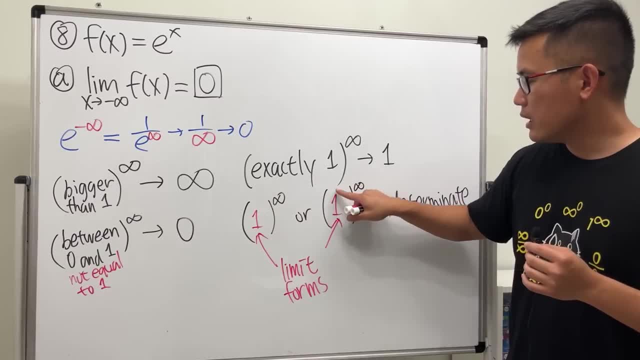 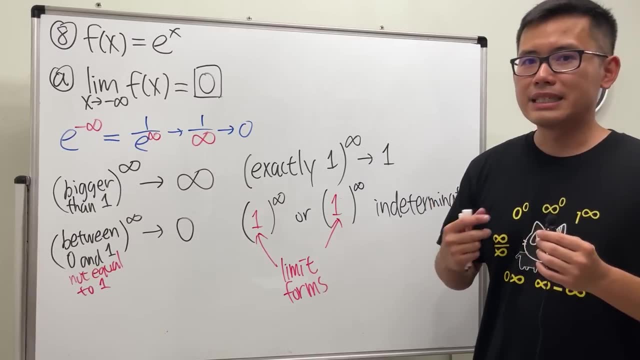 of this is that a lot of times we don't even put a plus or minus. That's why you see my shirt right here. We have a one to the infinity's power. A lot of times it's misunderstood that, hey, it shouldn't just be equal. 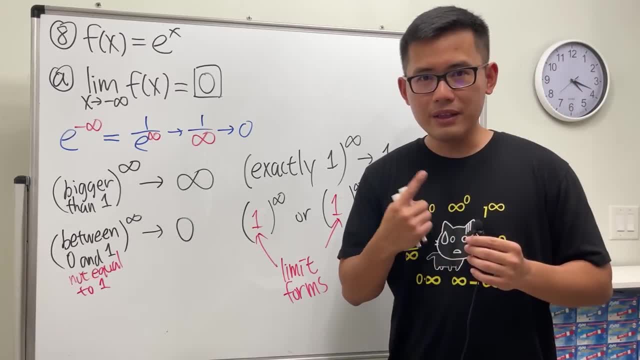 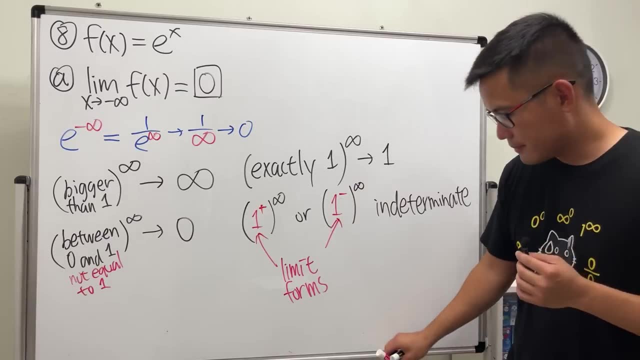 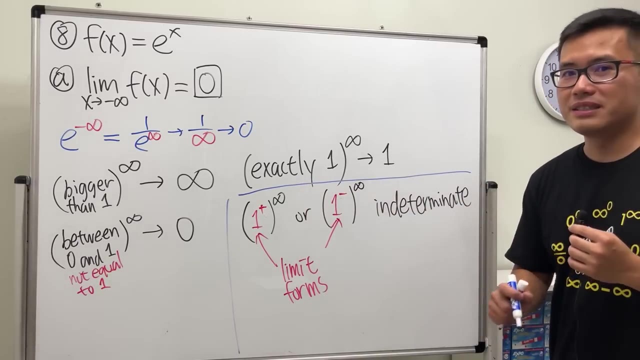 to one. No, no, This right here, this one, it's a limit form, meaning that it's technically saying one plus or one minus. So this right here, it's one of the most confusing part, And I would like to just give you guys an example before we go. 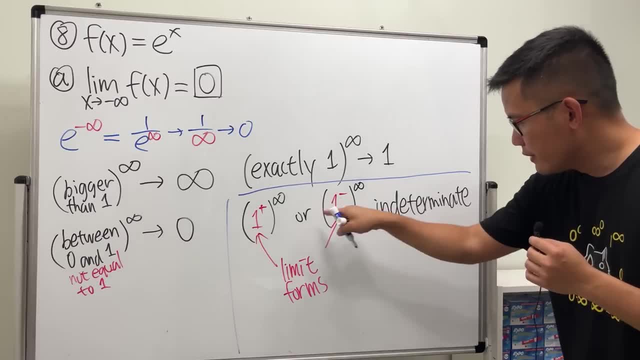 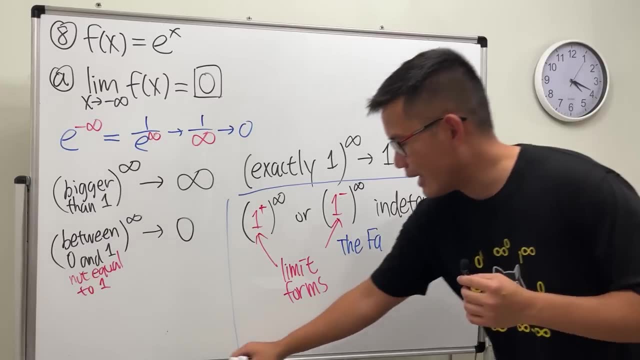 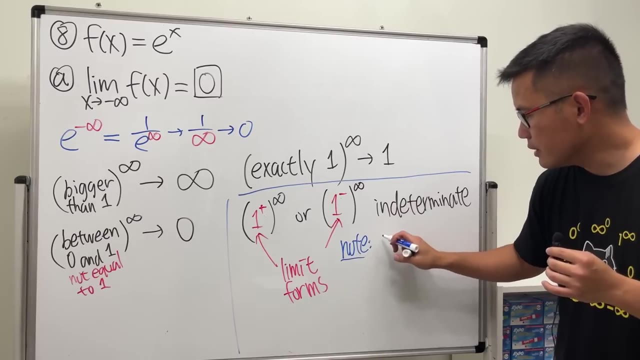 especially we're talking about e to the x power right. So the famous example for this one is: this: is called the fact. Well, actually, no, I'm not going to tell you guys the secret weapon yet, I'm just going to put down a note. 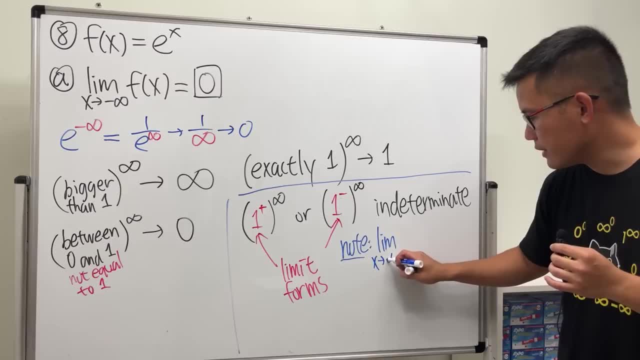 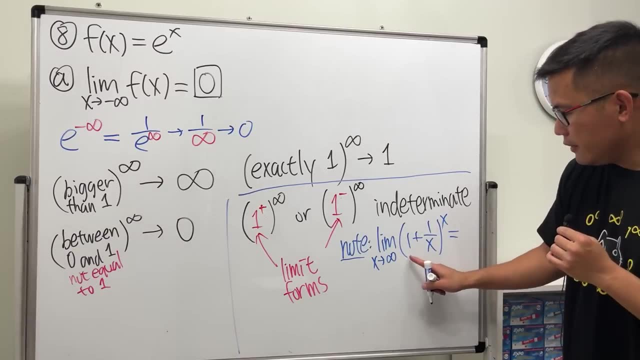 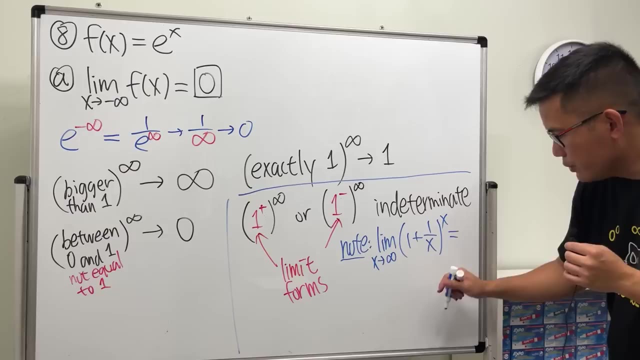 If we have the limit as x approaching infinity, one plus one over x to the x power. Check this out. If we put infinity to here and then just worked out like that, do this kind of thing, We are going to get one plus one over infinity. 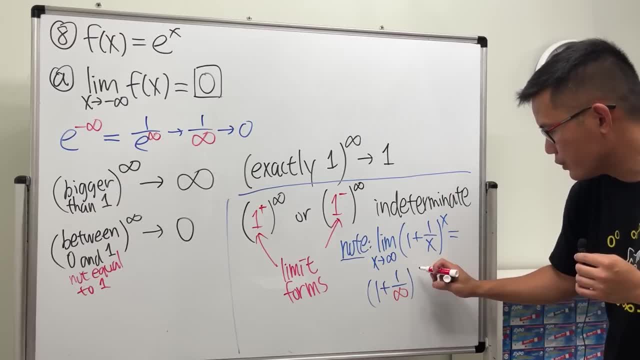 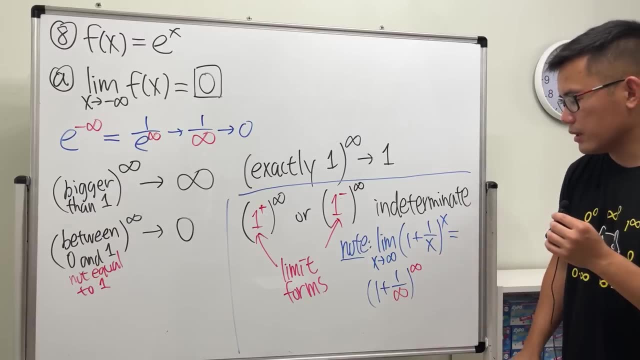 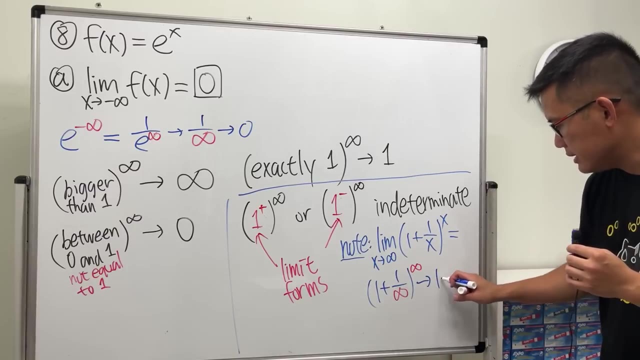 Right, And here we get infinity. and then to the infinity's power. Now I'm going to kind of argue like we'll reason things out along the way. One over infinity is zero, So this right here is approaching one plus zero. and then to the infinity's power. 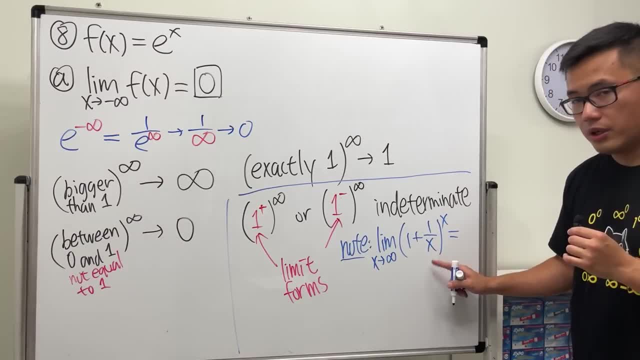 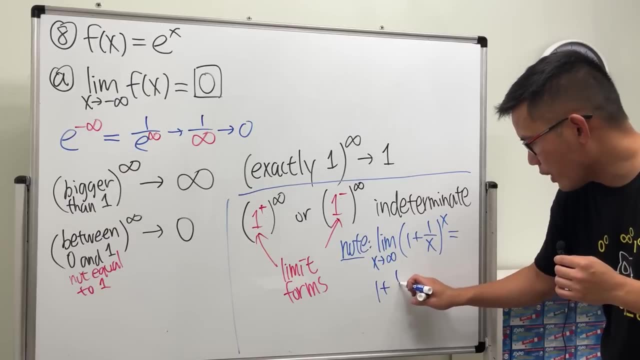 check this out. If we put infinity to here and then just work it out like that, do this kind of thing, we are going to get 1 plus 1 over infinity. right, Put this in here, we get infinity, and then to the infinity's power. 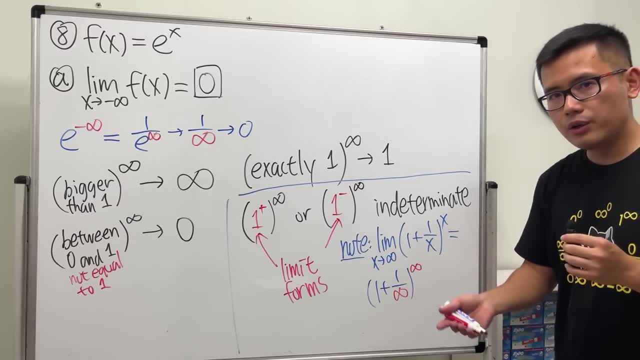 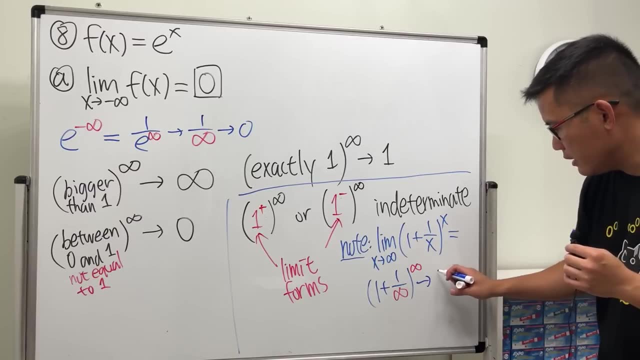 Now I'm going to kind of argue like we'll reason things out along the way: 1 over infinity is 0, so this right here is approaching 1 plus 0, and then to the infinity's power right. 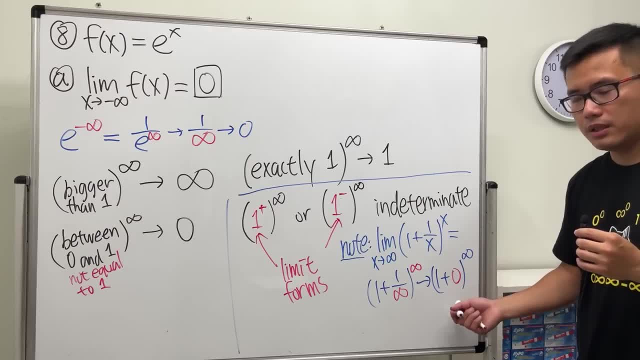 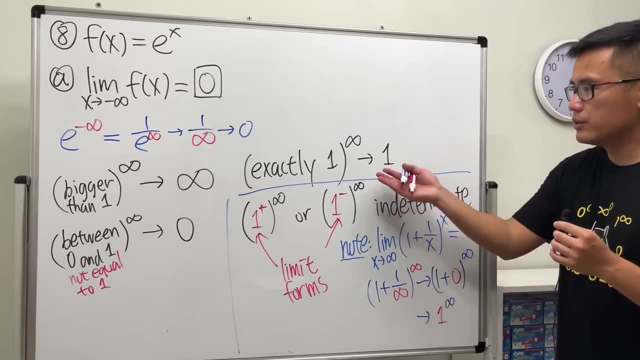 And then what's 1 plus 0?? 1 plus 0 is 1.. So this right here is approaching 1 to the infinity's power, right, And now it's like contradicting. I'm saying that this right here is exactly 1 to the infinity. 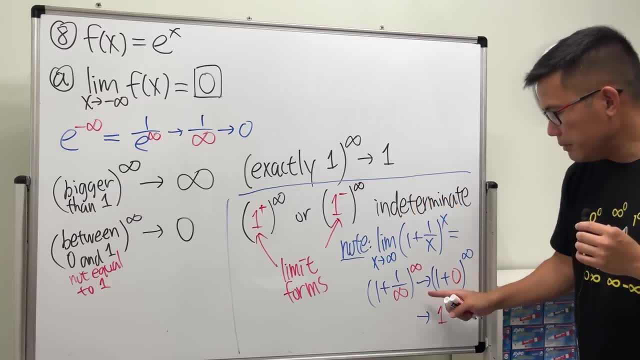 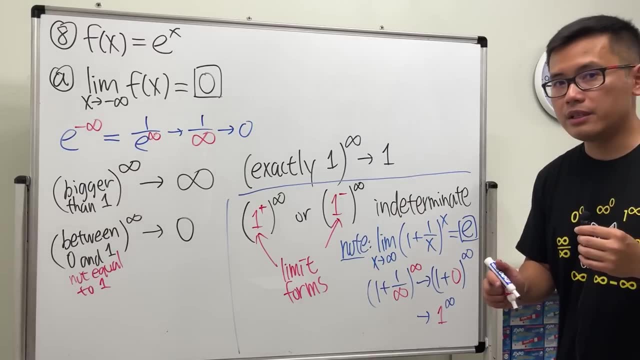 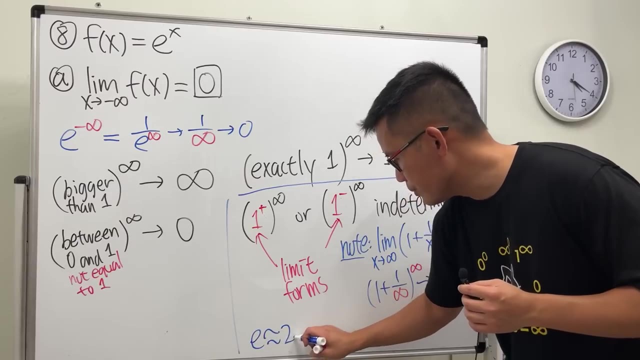 No, what am I talking about? Let me tell you This particular limit. the answer that we get is actually e, which is about 2.718-ish. okay, So I'm just going to write this down right here: e is about 2.718.. 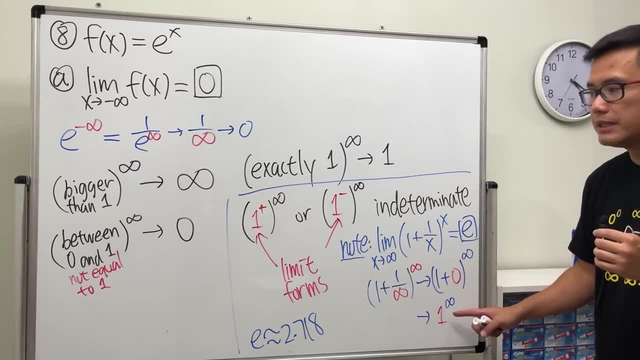 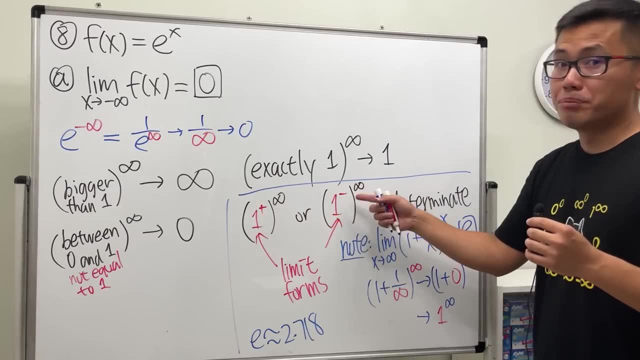 And again, if you look at this, why this is an indeterminate form. It's because we just write it down as 1 to the infinity, but really it means the limit form, either 1 plus or 1 minus. Why? 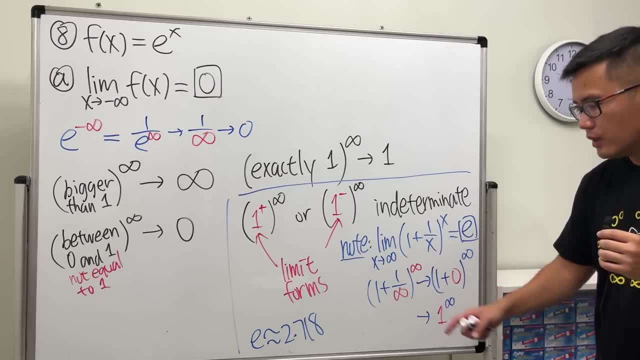 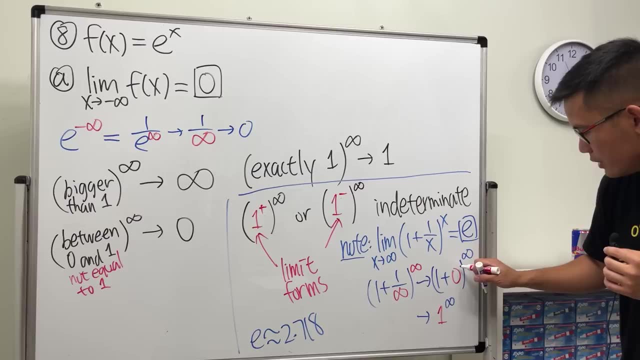 Because this 0 here it's not exactly 0.. 1 divided by infinity, The value is not exactly 0.. The limit is 0.. So technically you should say this is like 0 plus Just a little bit bigger than 0.. 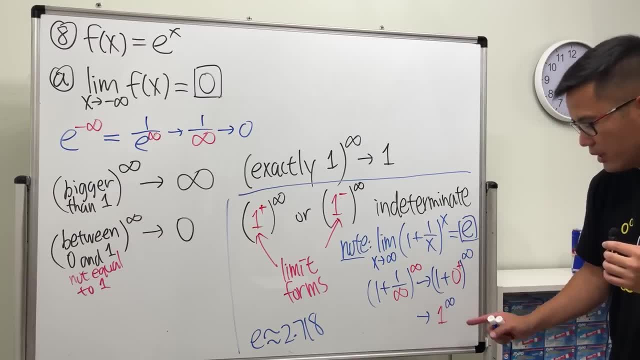 That kind of thing. And then right here we have 1 to the infinity's power. This is technically 1 plus and then raised to the infinity's power. Yeah, But unfortunately when we're talking about the limit form, nobody writes it like this. 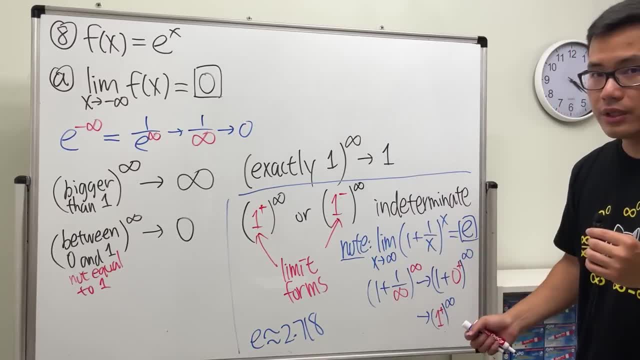 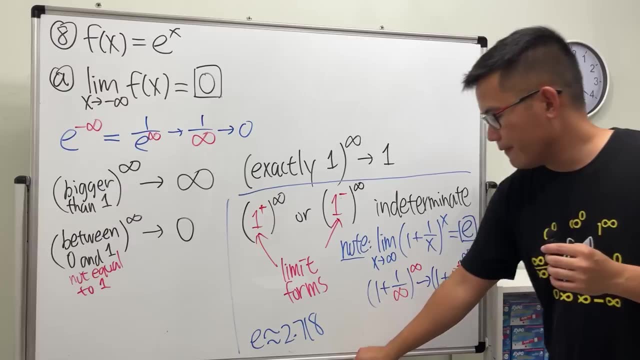 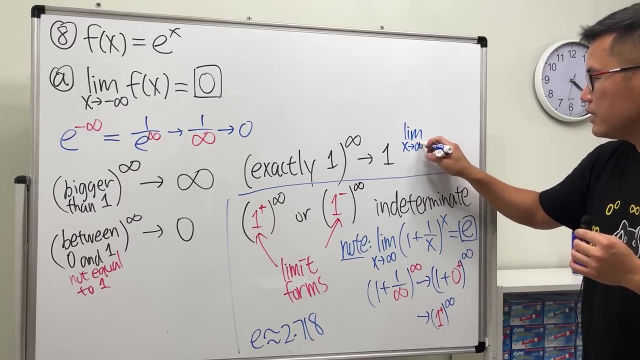 So you just have to be aware of this kind of situation, okay, And what I mean by exactly equal to 1 is that if today- I have a very redundant example- let's say, if we have a limit as x approaching infinity, if we just have a solid 1, nothing else. 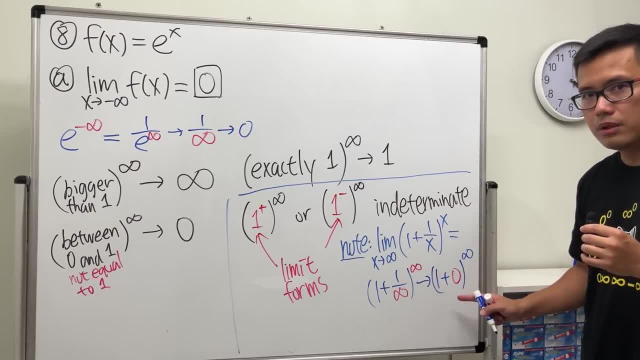 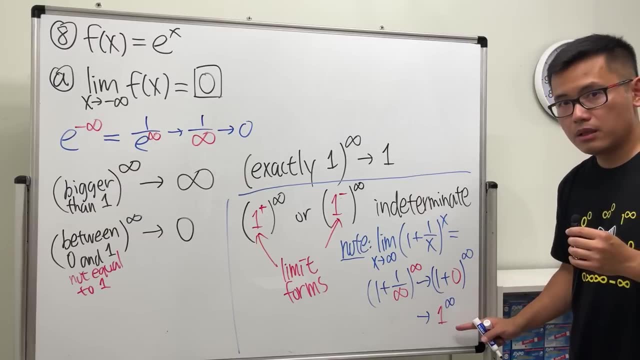 Right. And then what's one plus zero? One plus zero is one. So this right here is approaching one to the infinity's power. Right, And now it's like contradicting. I'm saying that this right here is exactly one to infinity. 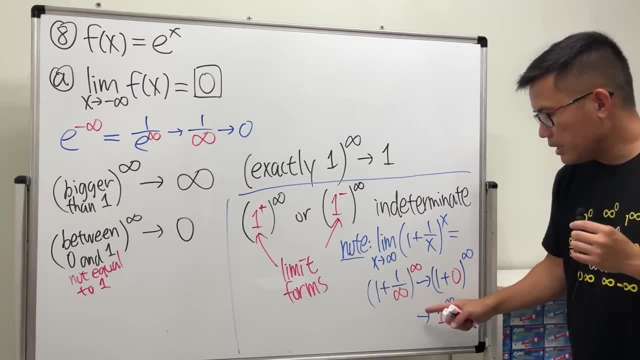 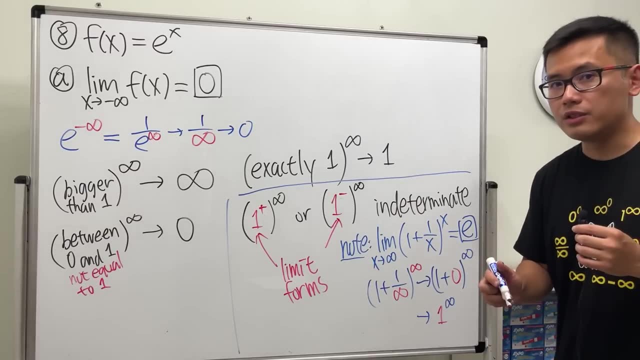 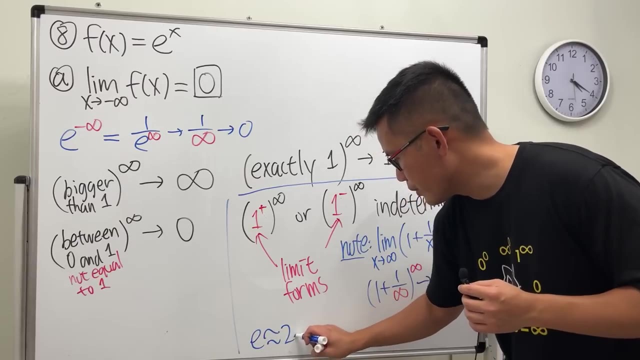 No, What am I talking about? Let me tell you this particular limit. the answer that we get is actually E, which is about two point seven, one eight-ish, OK, so I'm just going to write this down right here: E is about two point seven, one eight. 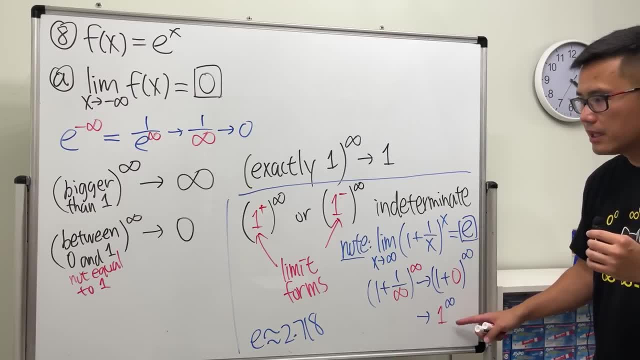 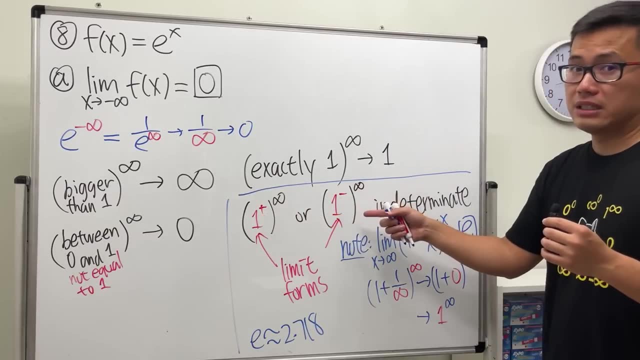 And again, if you look at this, why this is the indeterminate form? it's because we just write it down as one to the infinity, But really it means the limit for either one plus or one minus. Why? Because this zero here it's not exactly zero. 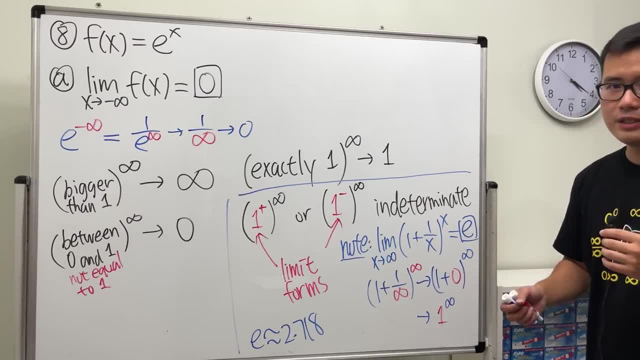 One divided by infinity. The value is not exactly zero, The limit is zero. So technically you should say this is like zero plus just a little bit bigger than zero, that kind of thing. And then right here we have one to the infinity's power. 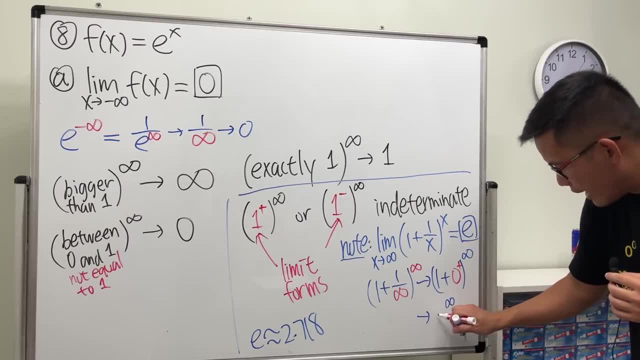 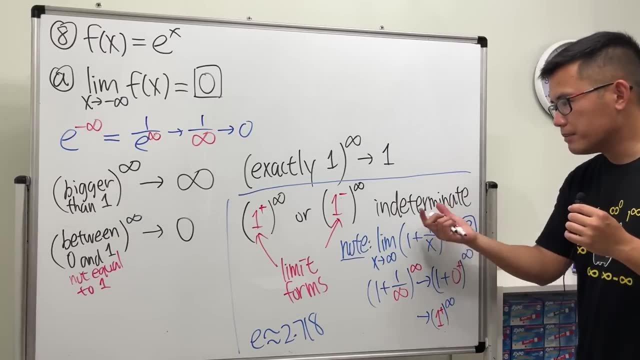 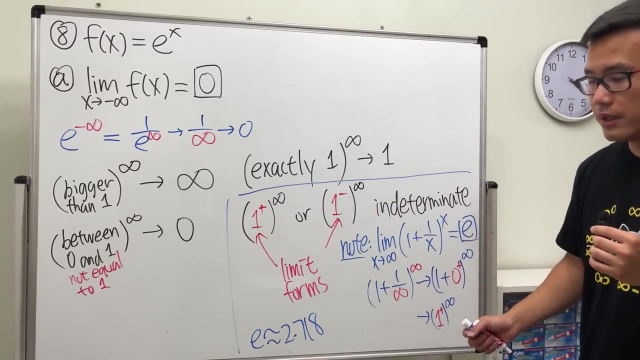 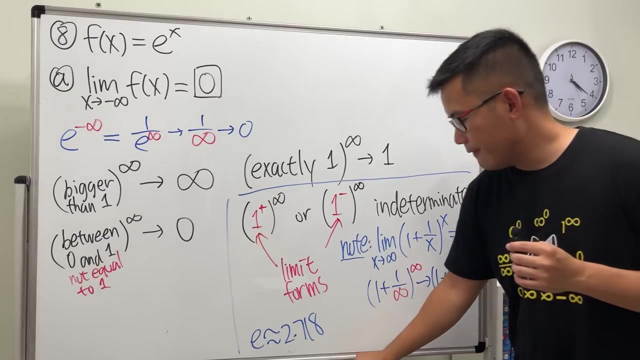 This is technically one plus and then raised to the infinity's power. Yeah, But unfortunately, when we're talking about the limit form, nobody writes it like this. So you just have to be aware of this kind of situation. OK, And what I mean by exactly equal to one is that if today I have a very 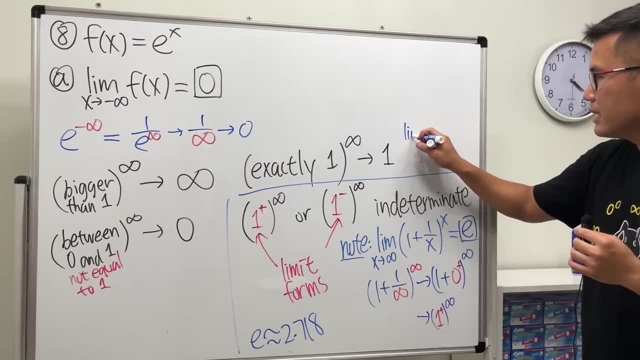 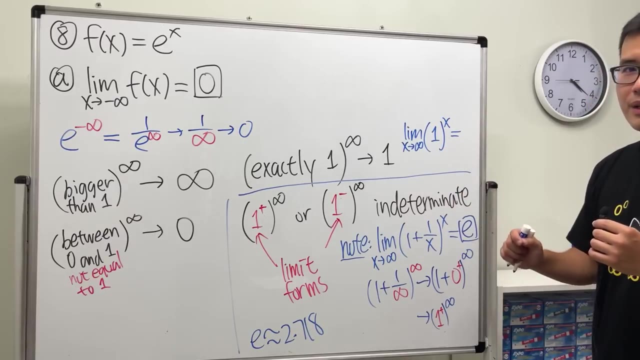 redundant example. let's say, if we have a limit as x approaching infinity, if we just have a solid one, nothing else, and then raised to the x power- you see, I'm not adding anything, just one, just one- And then to the infinity's power. the answer for this, right here, is equal to one. 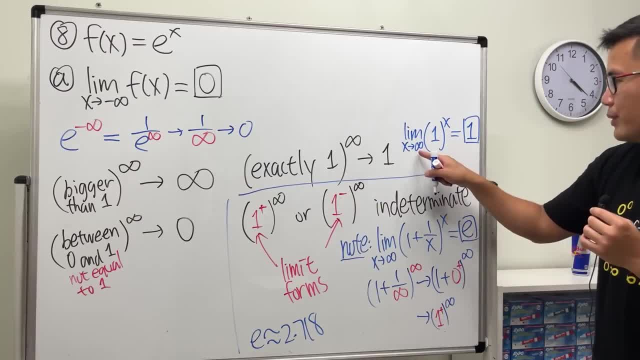 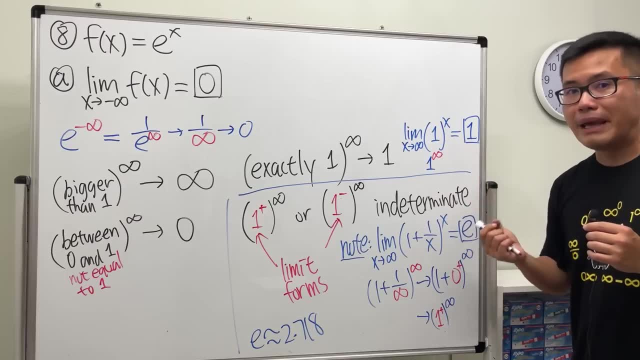 Why? Because the base is exactly equal to one, And if you put infinity to here, you really get one to the infinity. But in this case you have to really understand what the base is. That's what I'm trying to say. 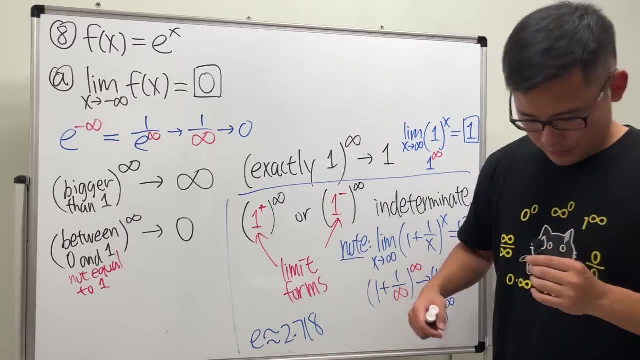 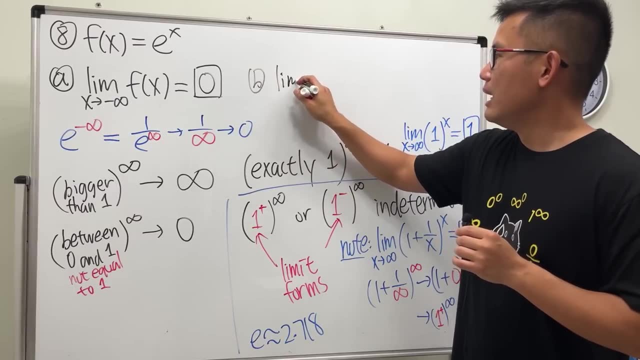 All right, So keep all these things in mind. Well, I'm not looking at my show, I'm looking at the question. OK, That's part A. Now let's look at part B. Limit x approaching zero. f of x. 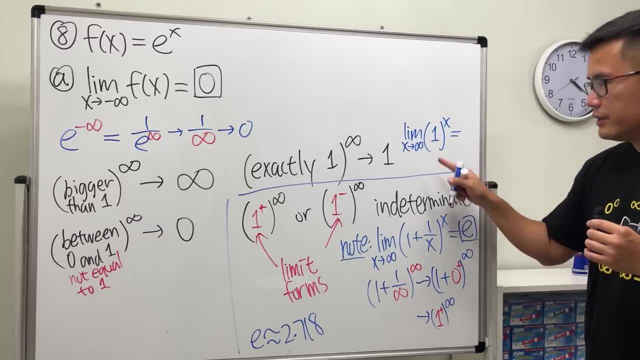 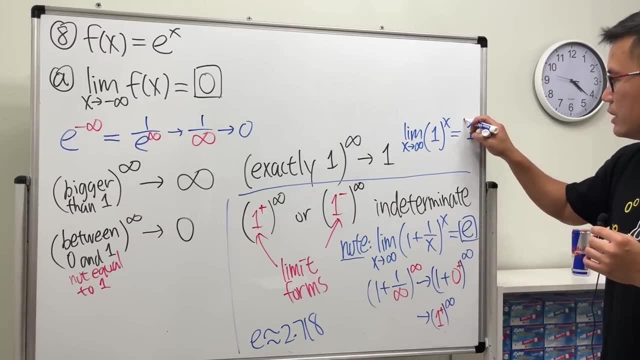 and then raised to the x power. you see, I'm not adding anything, just 1., Just 1.. And then to the infinity's power. The answer for this, right here, is equal to 1.. Why? Because the base is exactly equal to 1.. 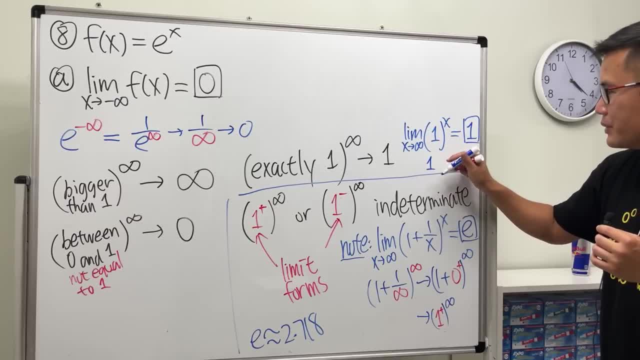 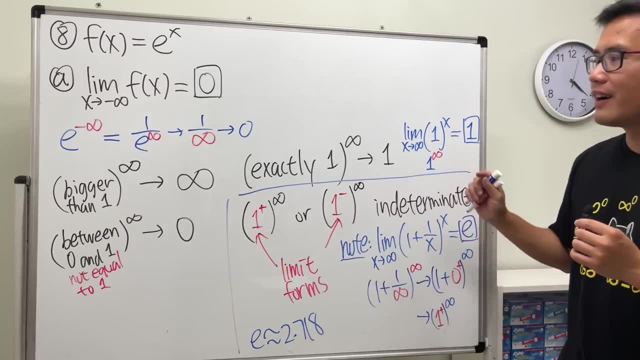 And if you put infinity to here, you really get 1 to the infinity. But in this case you have to really understand what the base is. That's what I'm trying to say. All right, So keep all these things in mind. 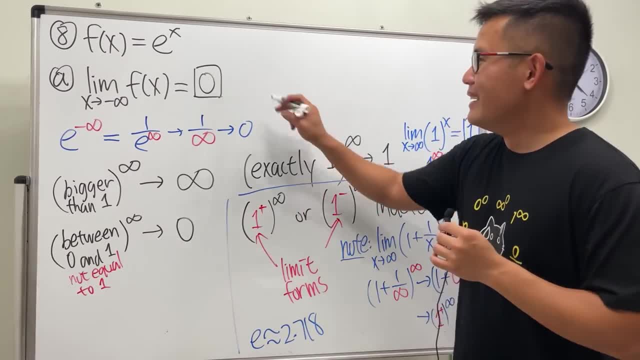 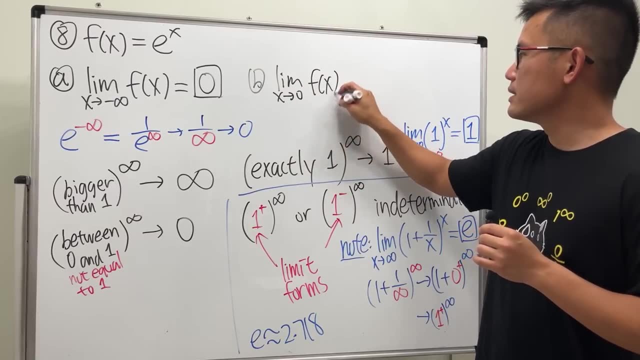 Well, I'm not looking at my show, I'm looking at the question. Okay, That's part A. Now let's look at part B. Limit x approaching 0.. f of x. This is nice, We can put 0 into the x value here. 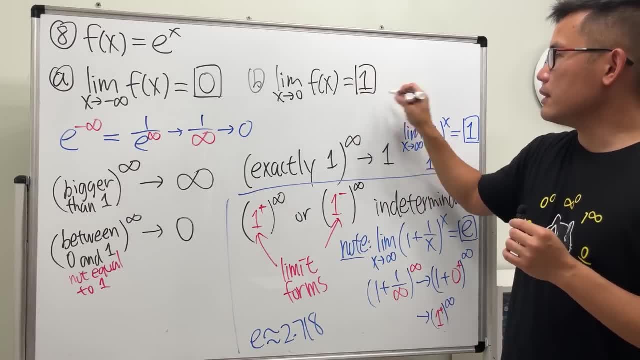 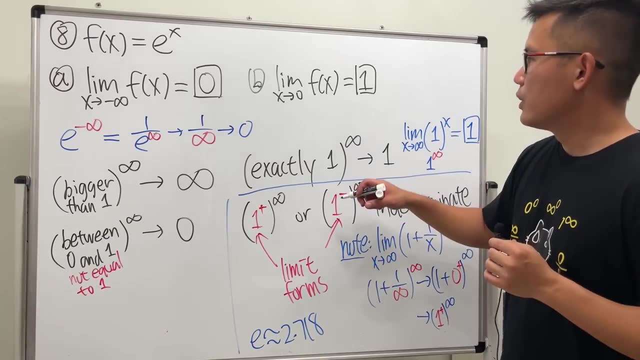 e to the 0's power is just 1.. So the answer is just 1. Done. And then, lastly, let me see if I can fit in part C. Okay, I'll fit in part C right here, If we have the limit x approaching infinity. 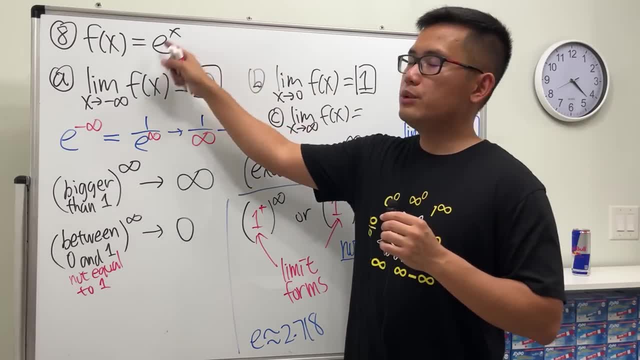 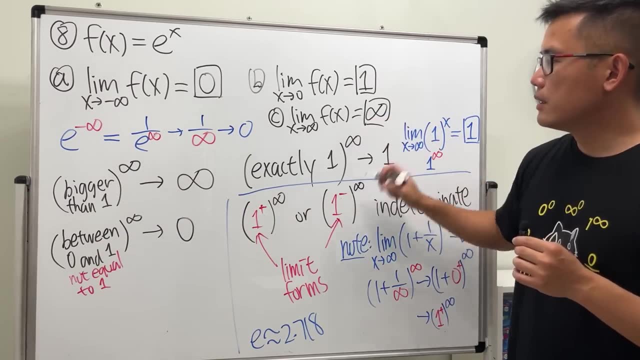 Per our discussion. if we put infinity into here- e to the infinity, e is bigger than 1, right To the infinity's power, This right here will give us infinity. So let me just kind of make a quick divider. 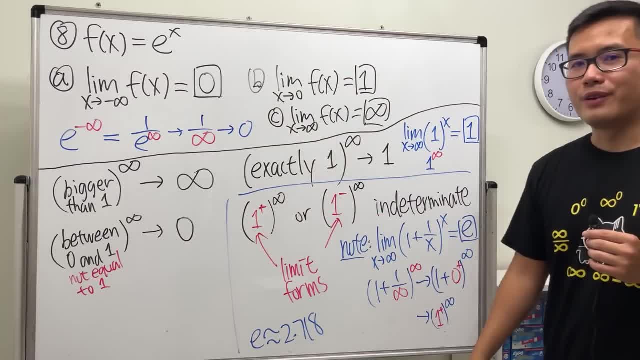 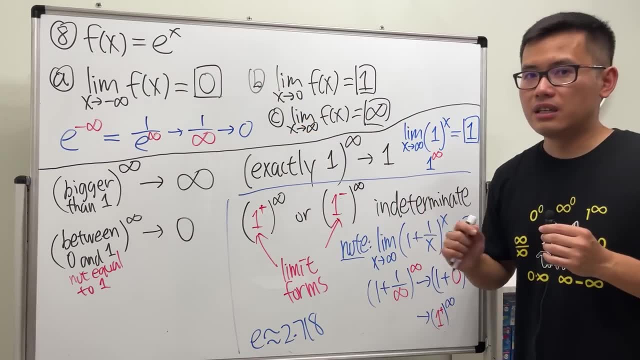 a, b, c and then these are the nodes. Now, what's going over here? Best of all, when we have a function, if we know the graph, we can answer a lot of the limits question without worry. So let me give you guys the picture. 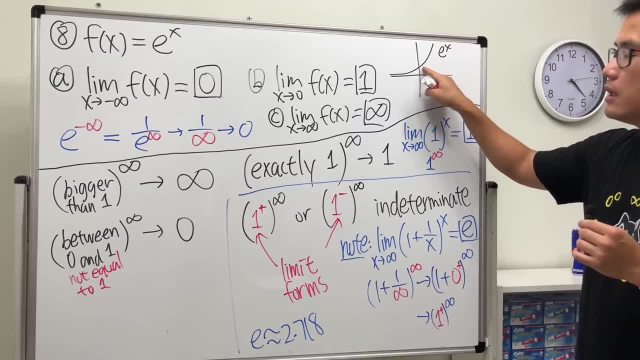 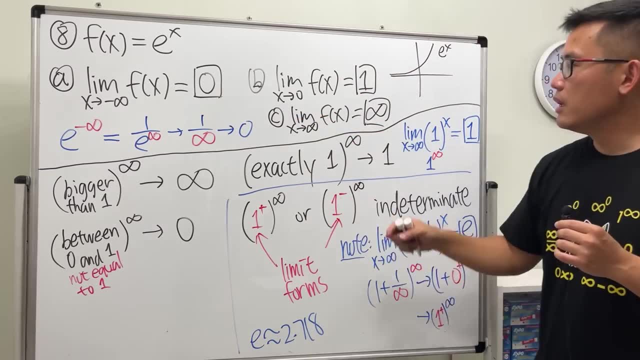 e to the x looks like this: So x approaching infinity, So x approaching infinity, Negative infinity, all the way to the left y value approaching 0.. x approaching 0, this y value is 1.. It's nice and continuous, it's just 1.. 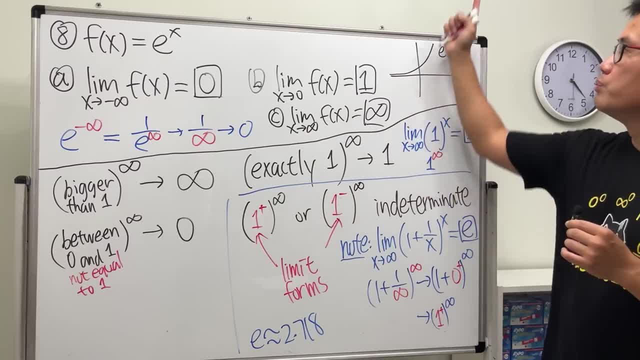 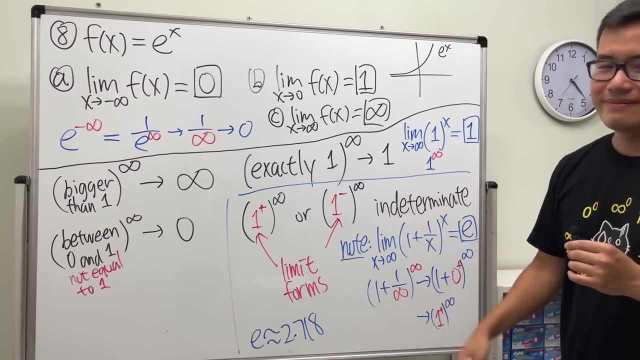 x approaching positive infinity all the way to the right y value, goes up to my ceiling, to the 3rd or the 4th, I don't know- 10th floor. It's infinity. So, ladies and gentlemen, that's number 10.. 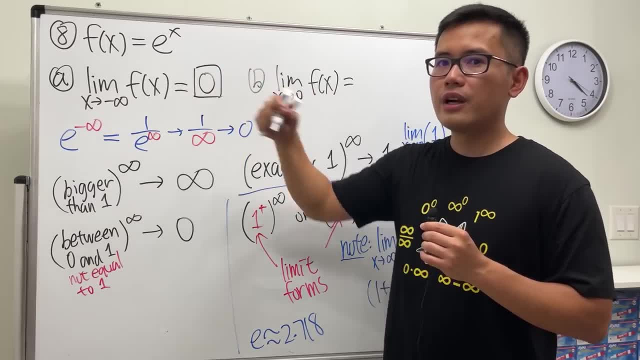 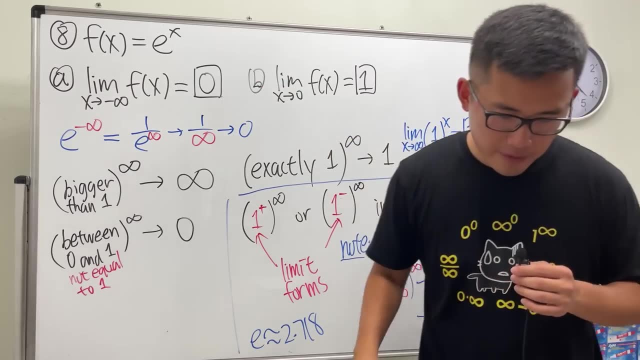 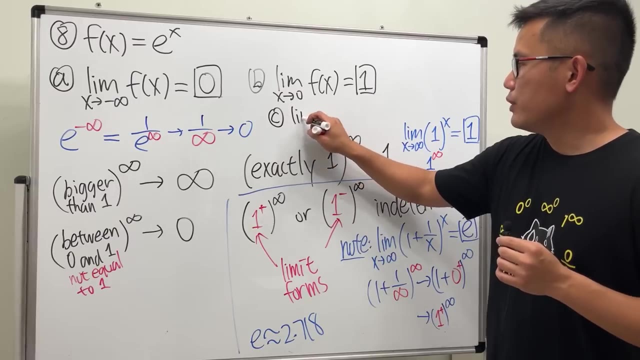 This is nice. We can put zero into the x value here. E to the zero's power is just one, So the answer is just one Done. And then, lastly, let me see if I can fit in part C. OK, I'll fit in part C right here, If we have the limit. 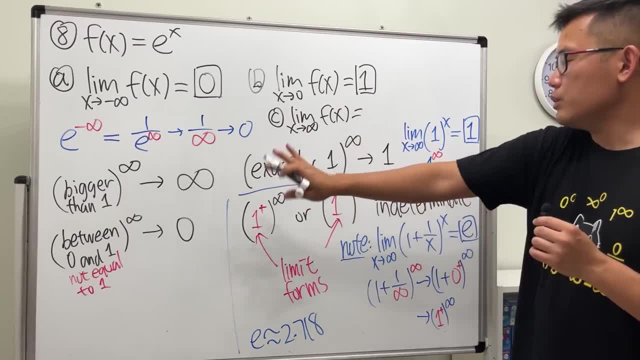 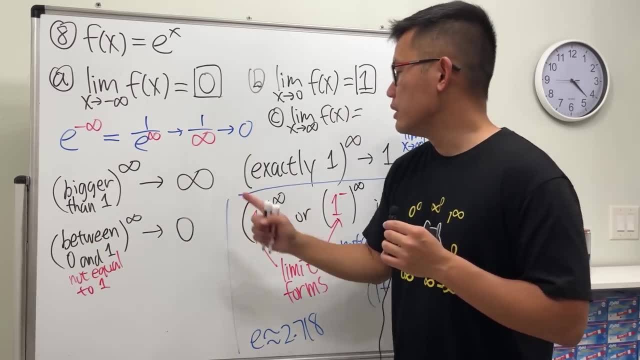 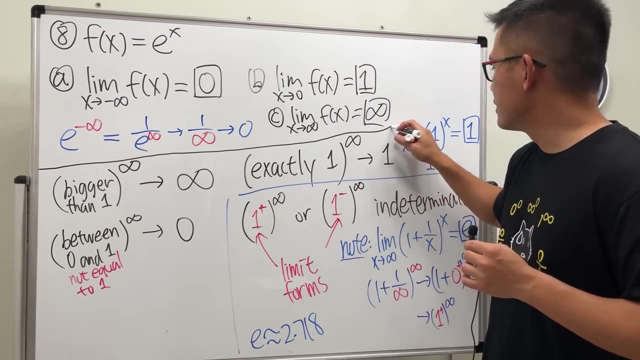 f of x approaching infinity. per our discussion, if we put infinity into here, e to the infinity, e is bigger than one right to the infinity's power. this right here will give us infinity. So let me just kind of make a quick divider. 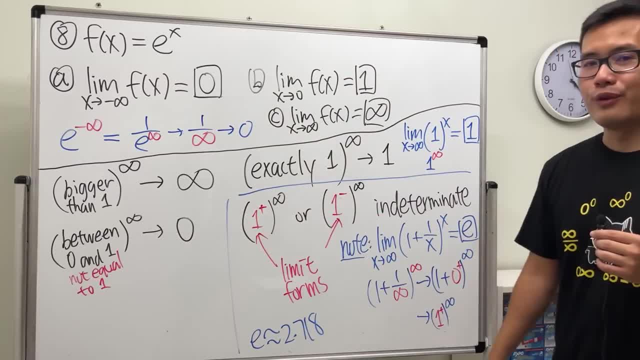 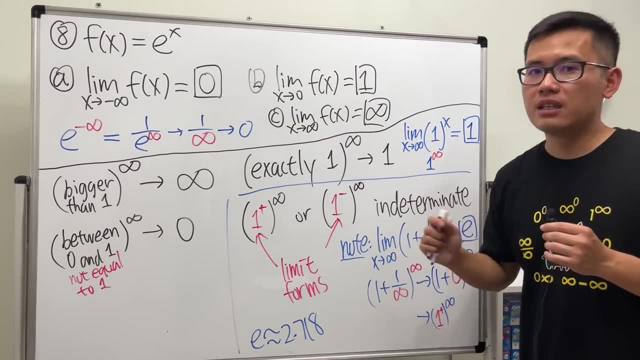 A, B, C and then these are the nodes that I was going over earlier. Best of all, when we have a function, if we know the graph, we can answer a lot of the limits question without worry. So let me give you guys the picture. 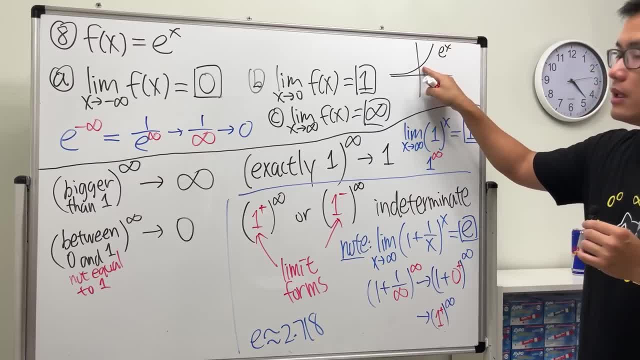 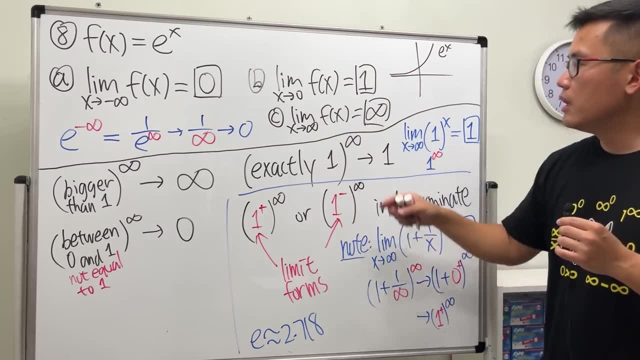 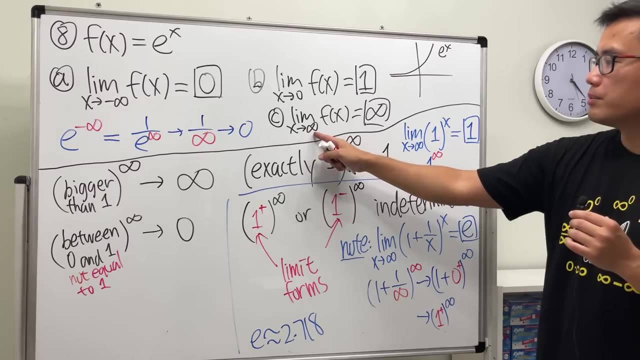 E to the x looks like this. So: x approaching infinity, negative infinity, all the way to the left, y value approaching zero, x approaching zero. This y value is one. It's nice and continuous, It's just one. x approaching positive infinity all the way to the right. y value goes up to my ceiling. 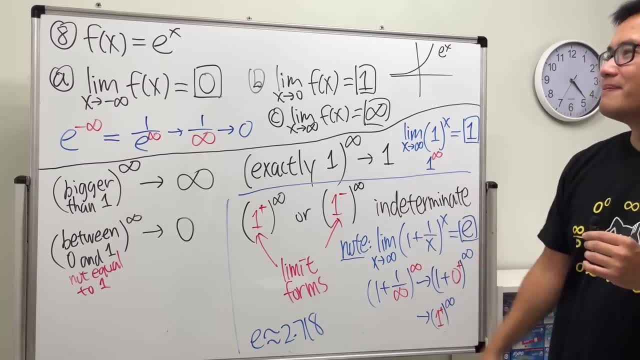 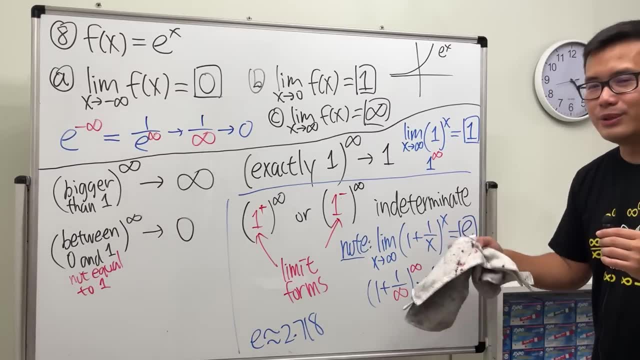 To the third or the fourth, I don't know- Tenth floor. It's infinity. So, ladies and gentlemen, that's number ten And, more importantly, please, please, please know this really, really well. All right, This is like the most asked question in any calculus class. 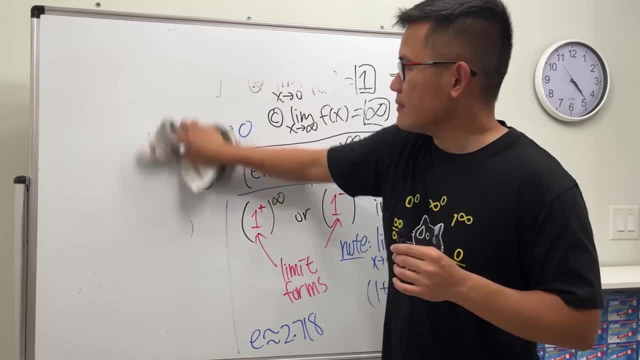 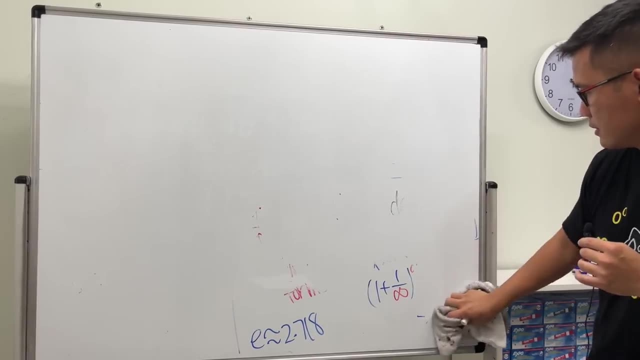 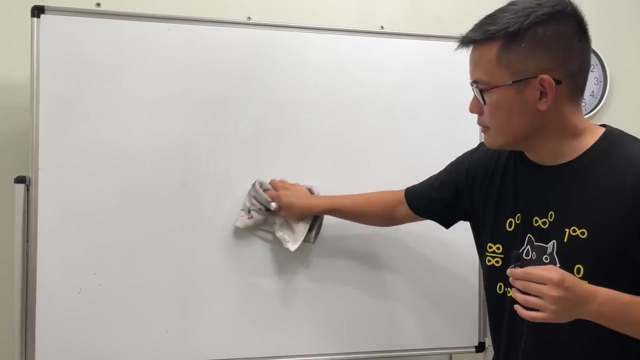 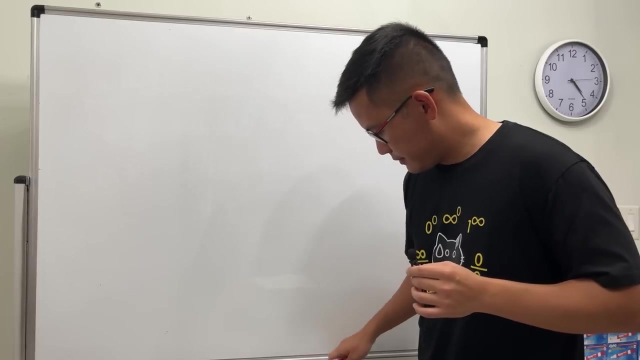 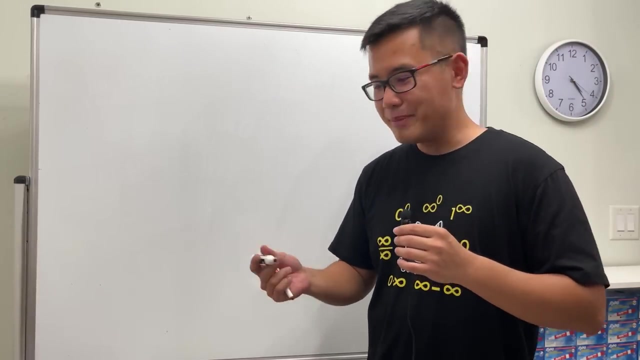 especially when we're talking about limits. Number nine, number 10.. I'm going to do like a function and it's in first again, So let's do. can number nine. Let's look at the function, Just tangent x, and Let's see. 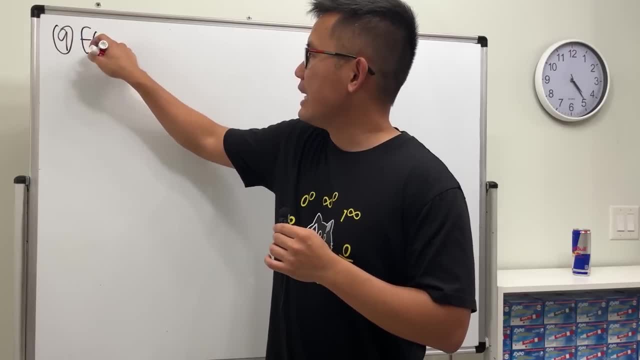 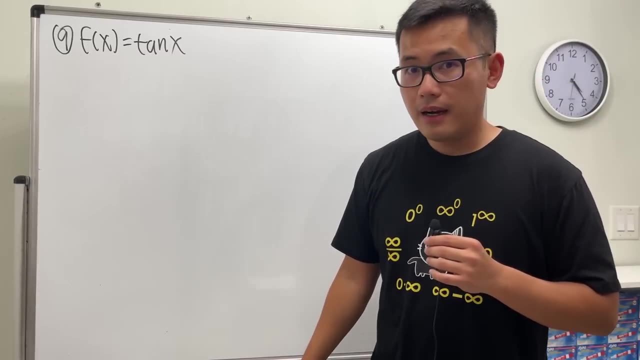 I'm going to write down A, B, C. let me look at the function- Just tangent x- and let me see what we can do. Let me just take the second to the right. So if I take this right, I'm going to take the third. 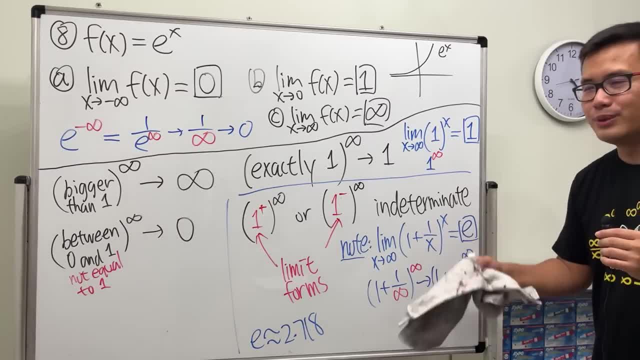 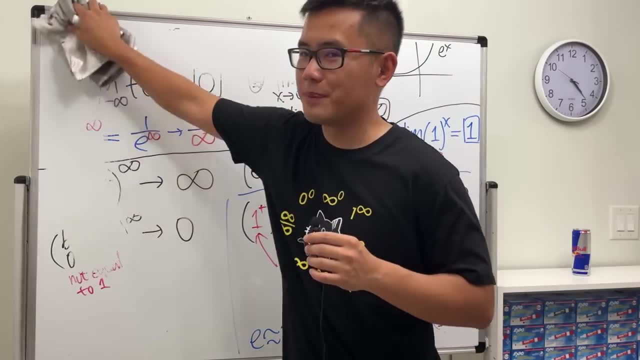 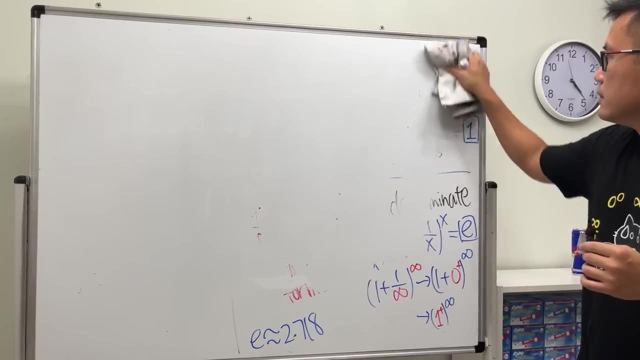 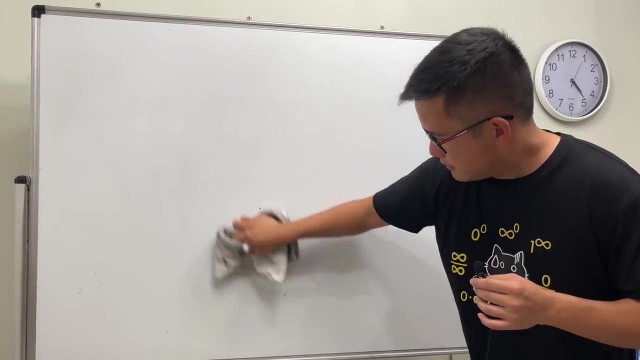 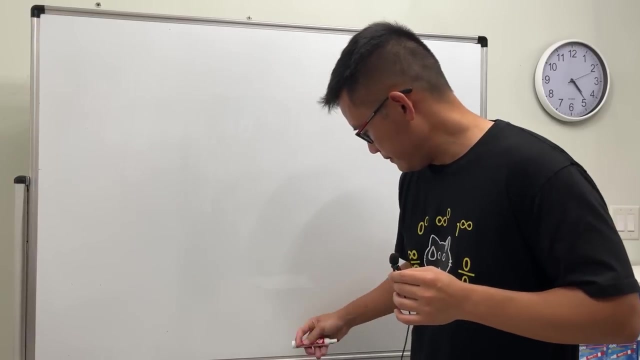 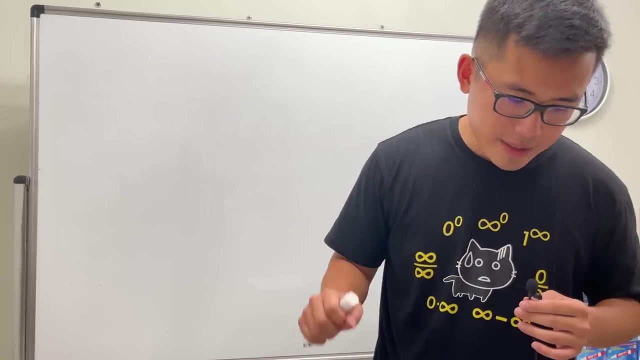 And, more importantly, please, please, please, know this really really well. All right, This is like the most asked question in any calculus class, especially when we're talking about limits. all right, number nine, number ten, i'm going to do like a function, and then it's inverse again. so 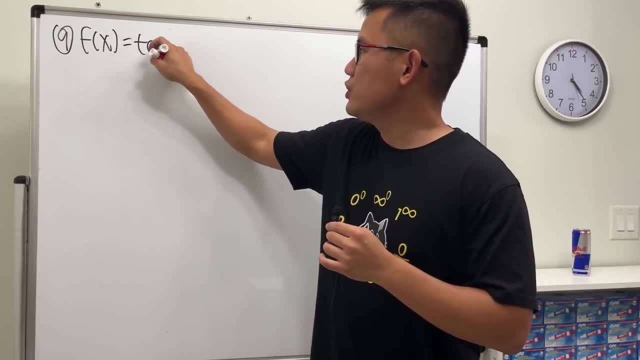 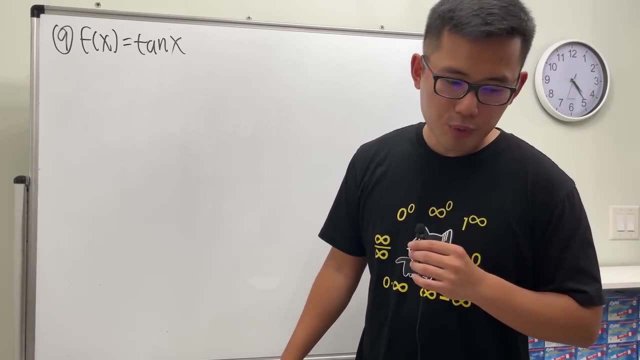 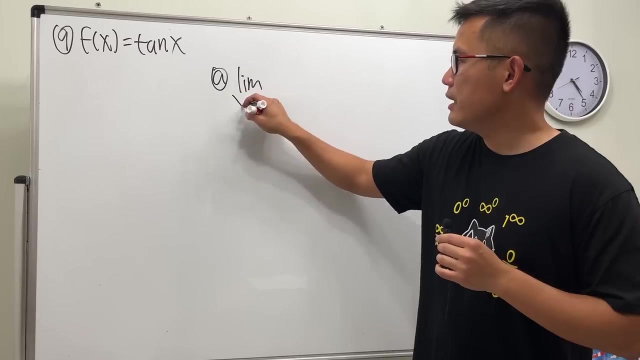 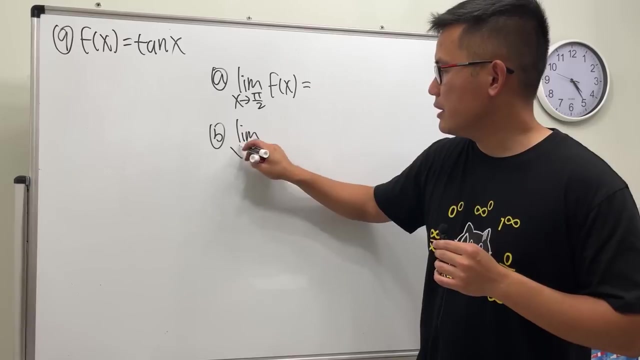 let's look at number nine. let's look at the function: just tangent x and um. let's see, i'm going to write down a, b, c and then i'm going to: let's put it down here. let's say: a- we have the limit x approaching pi over two f of x. b: limit x approaching infinity, f of x. 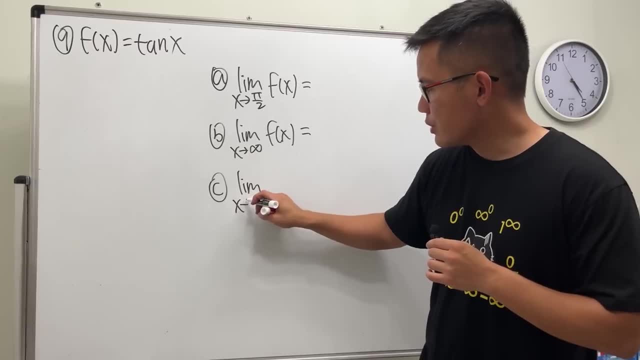 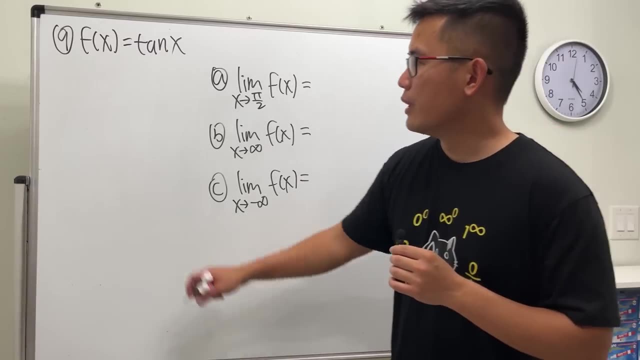 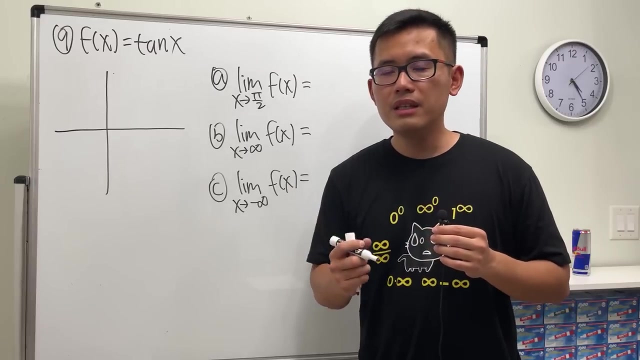 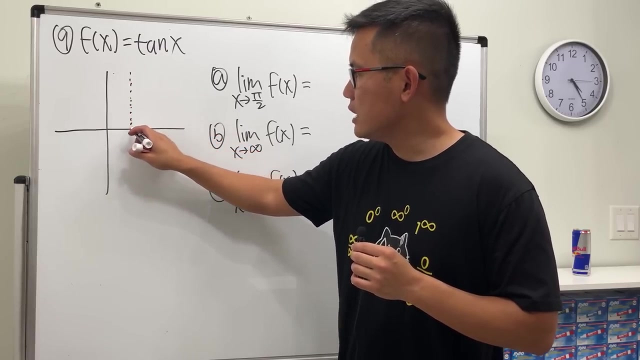 c limit. x approaching negative infinity. f of x ready cool inverse tangent, sorry, regular tangent. ladies and gentlemen, it looks like this: we have infinitely many vertical isotopes. the first one is right here. if you look at the positive x, for the first, pi over two, and then the next one is, you just add pi and you get three pi over two. 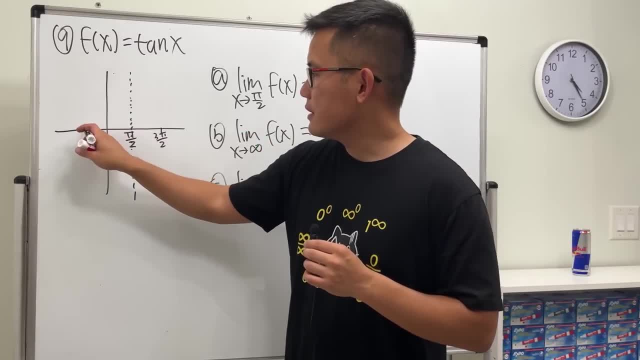 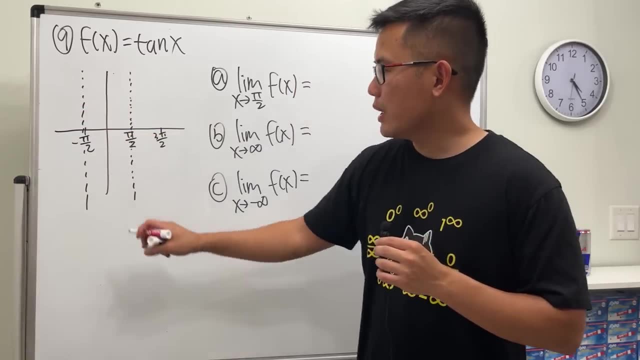 and so on, so on. so the one on the left, the first one here, is negative pi over two, and then so on, so on, so on, and then we are going to get a bunch of this. i'm just going to do this to make it more clear. 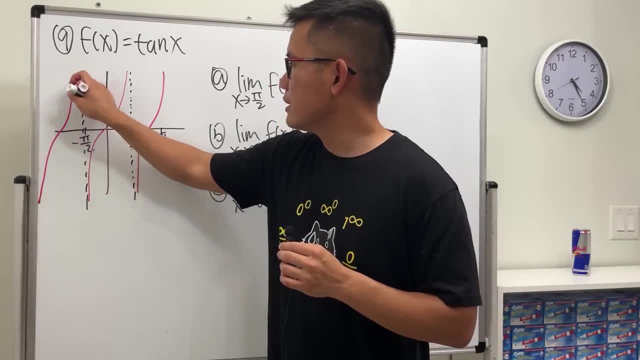 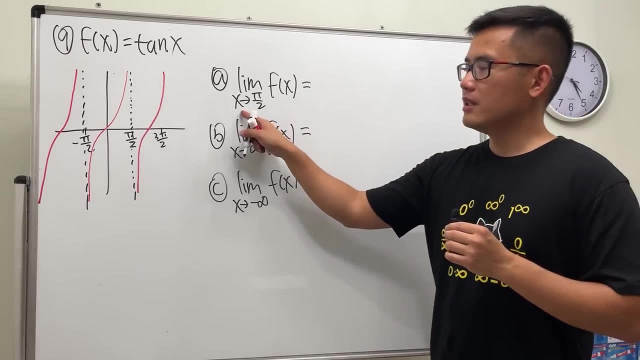 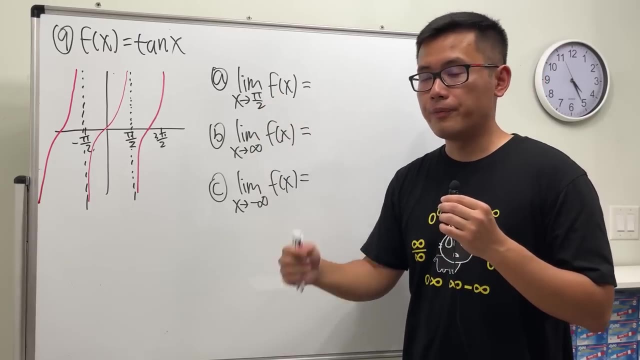 right. so bunch of this, one of the graphs that you should definitely have seen back in your pre-calculatory class. and, with that being said, let's look at the first limit as x approaching pi over two. we do not have the plus, we do not have the minus, so we do both when x is approaching. 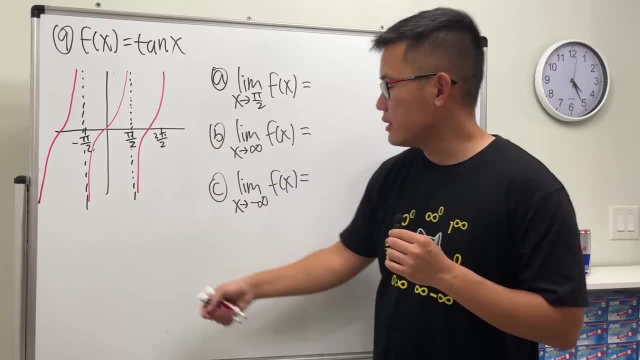 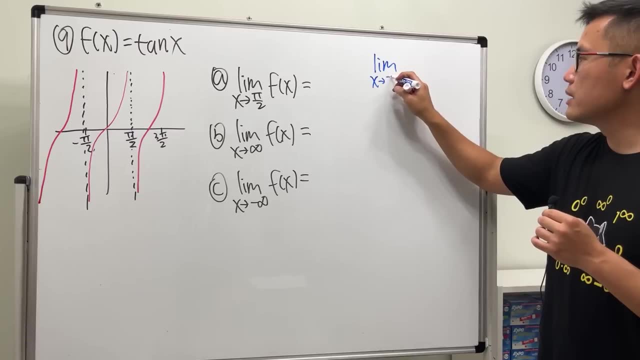 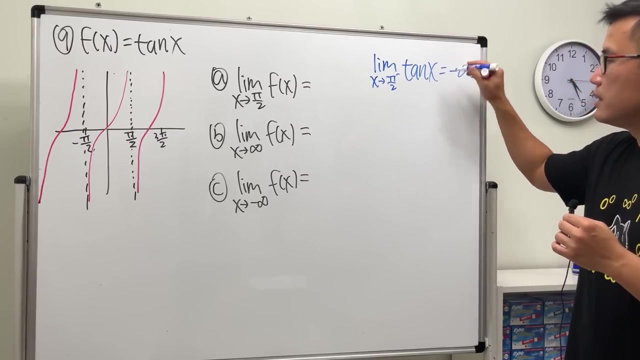 pi over two from the right we get negative infinity. so let me just write this down here: if we have the limit as x approaching negative infinity, f of x, b limit x approaching negative, so pi over two minus of our function tangent x, this right here is negative infinity. 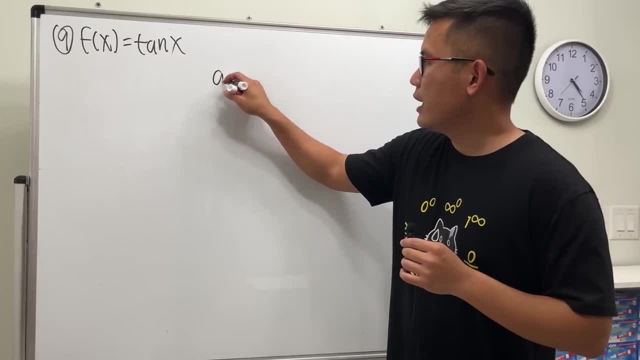 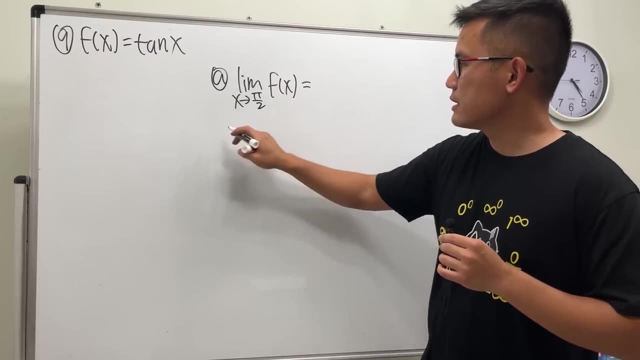 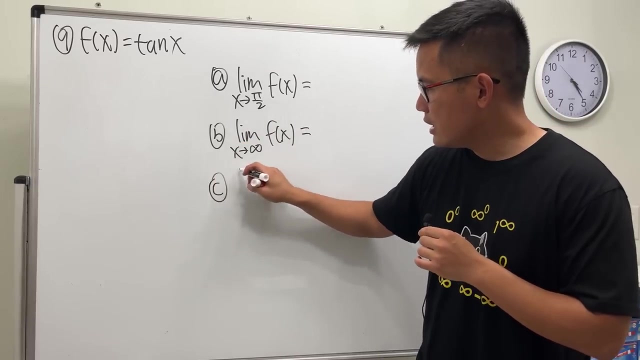 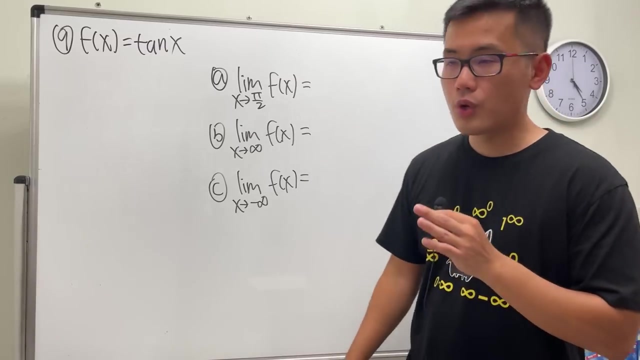 c. and then i'm going to- let's put it down here. let's say: a- we have the limit x approaching pi over 2 f of x. b. limit x approaching infinity f of x. c. limit x approaching negative infinity f of x. ready, cool inverse tangent, sorry, regular tangent, ladies and gentlemen. it looks like this: 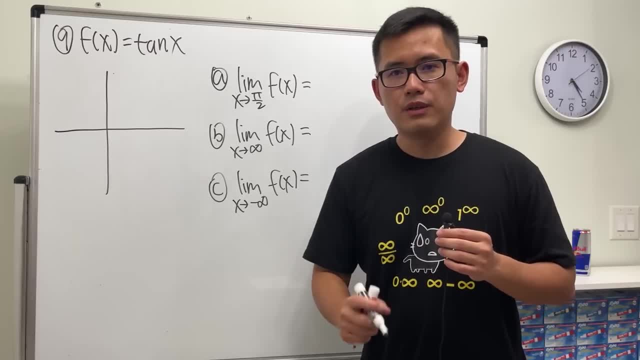 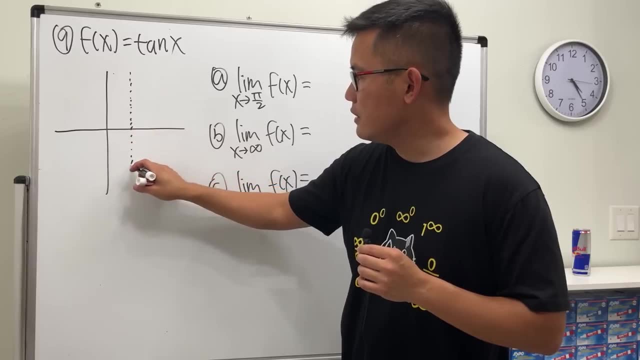 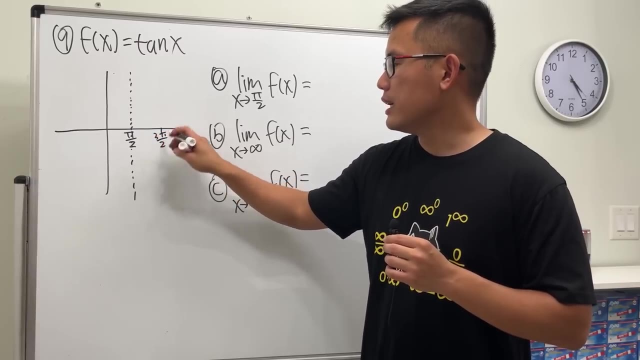 we have infinitely many vertical asymptotes. the first one is right here, if you look at the positive x for reverse pi over two. and then the next one is: you just add pi and you get 3 pi over 2, and so on, so on, so on the one on the left, the first one here: 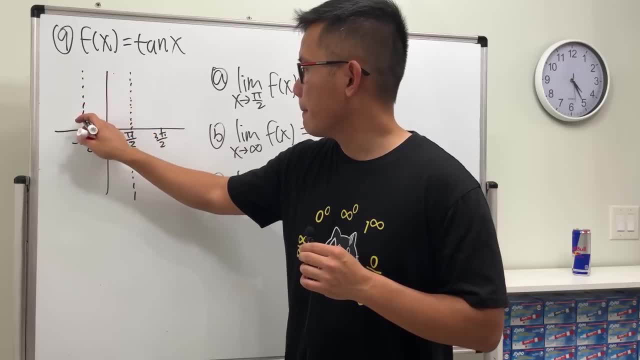 and then the second one is: you just add pi and you get 3 pi over 2, and so on, so on, so on. the one on the left, the first one here, is negative pi over two, and then so on, so on, so on, and then we are going to get bunch of this. 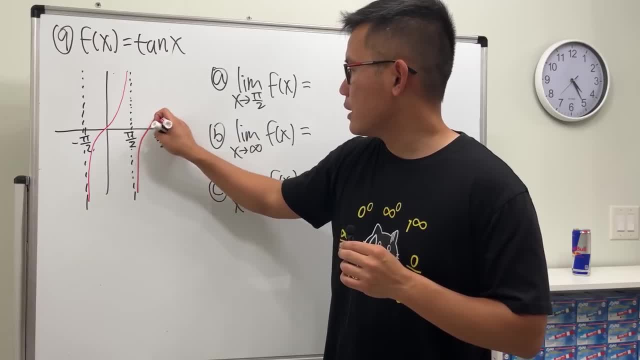 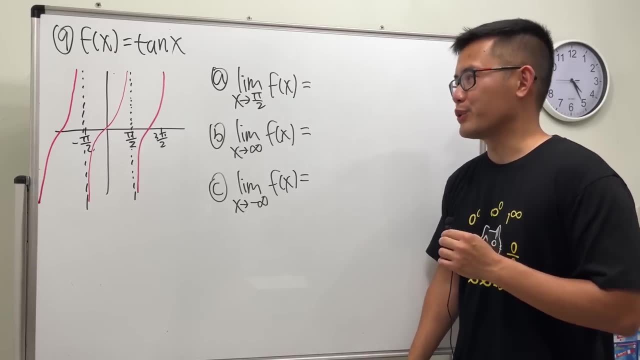 i'm just going to do this to make it more clear, right? so bunch of this, one of the graphs that you should definitely have seen back in your pre-calc or tree class, and, with that being said, let's look at the first limit as x approaching. 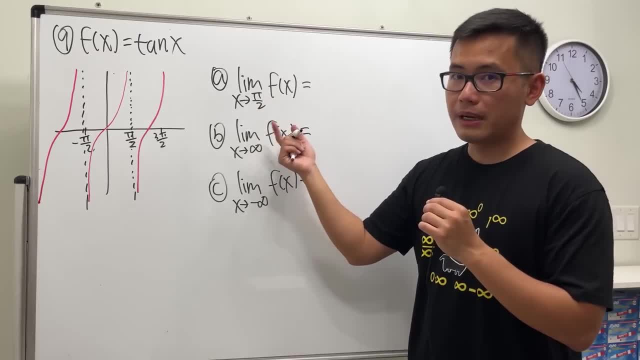 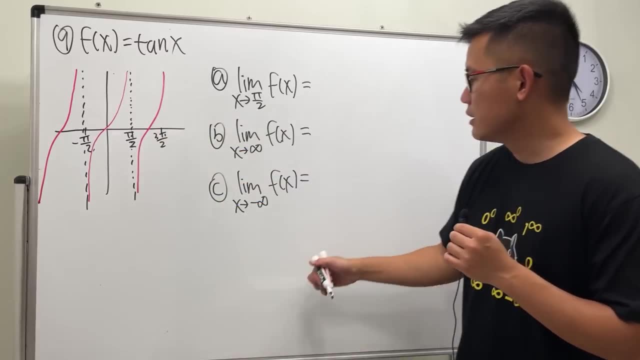 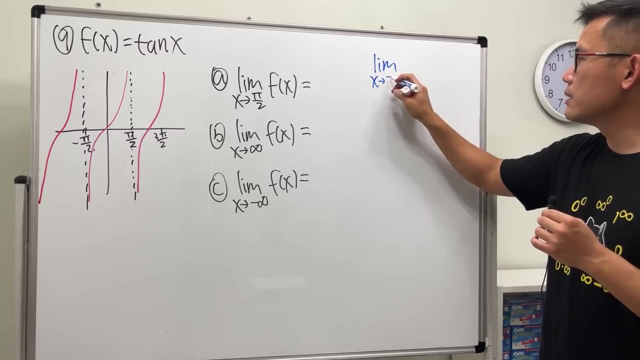 pi over 2, we do not have the plus, we do not have the minus, so we do both. when x is approaching pi over 2, from the right we can negative infinity. so let me just write this down here: if we have the limit as x approaching negative, so pi over 2 minus. 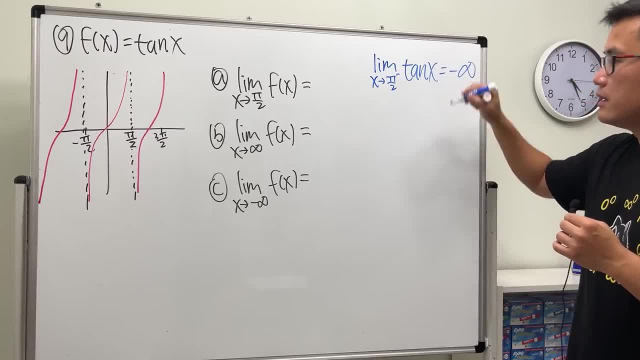 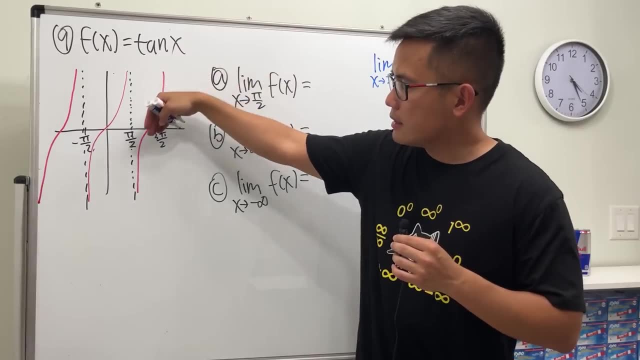 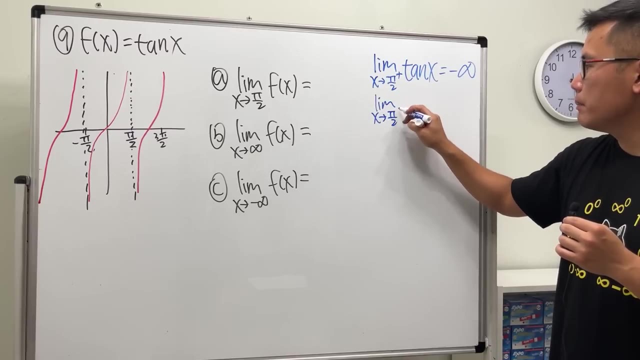 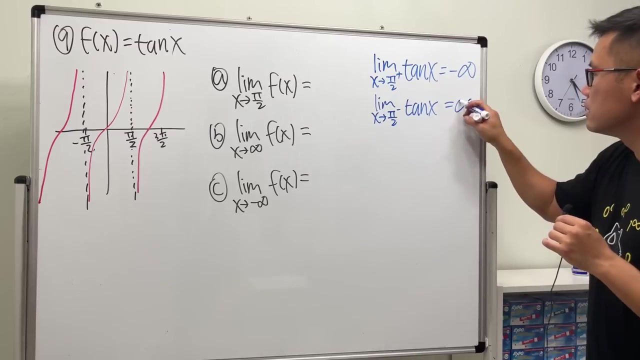 of our function. tangent x- this right here- is negative infinity. sorry, this should be a plus, sorry. pi over 2, plus. from the right the function goes straight down. and if we have the limit x approaching pi over 2 minus, tangent x- this right here- goes straight up. so positive infinity. they do not equal. 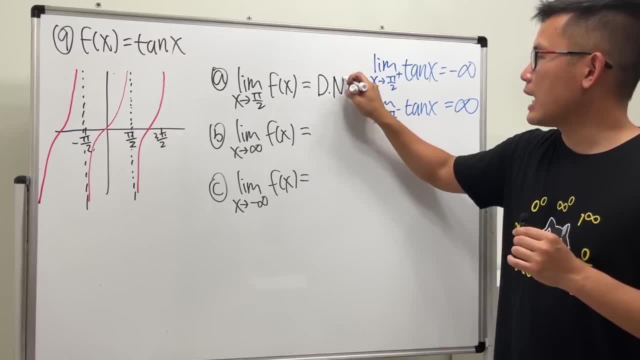 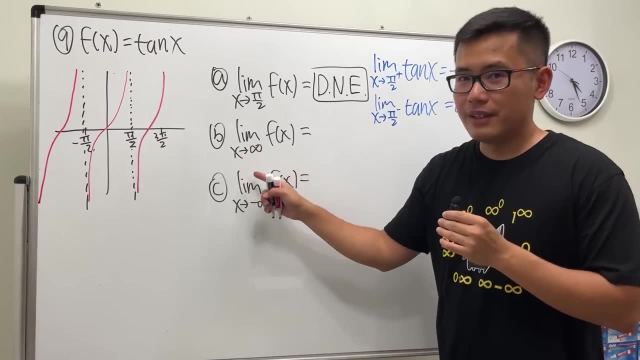 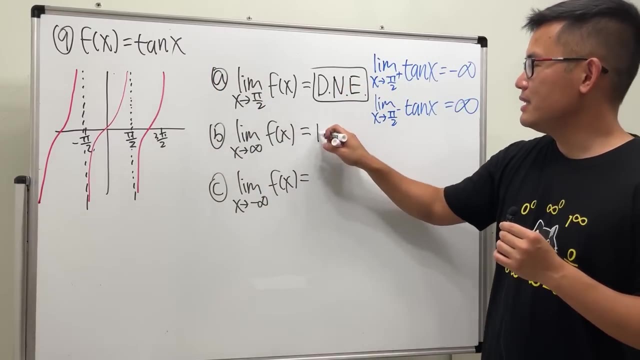 d and e i preferred with dots. you don't have to put down the dots anyway. limit as x approaching infinity. oh, this is crazy, just to keep on going. all right, the y how it does not approach to a certain number. so this right here. d and e, i prefer dots. similarly, x approaching negative infinity. 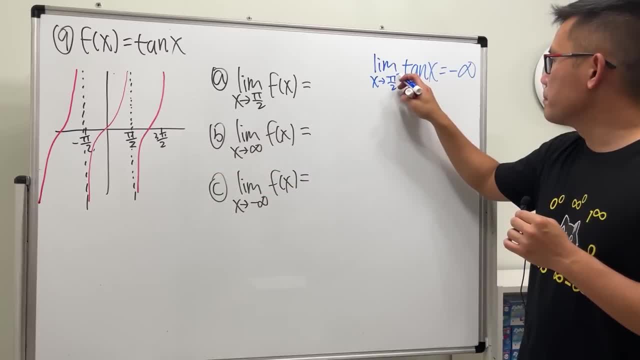 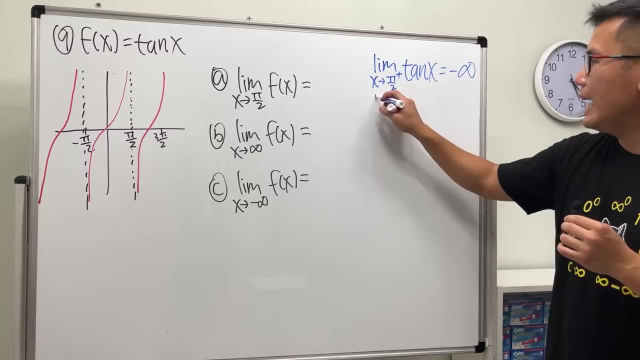 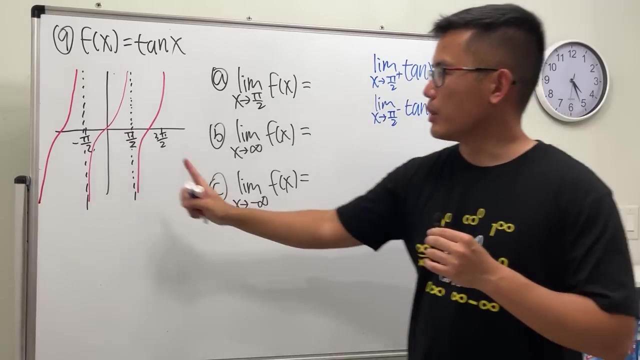 sorry, this should be a plus, sorry pi over two. plus. from the right the function goes straight down. and if we have the limit x approaching pi over two minus tangent x, this right here goes straight up. so positive infinity. they do not equal to negative infinity, so we get negative infinity. 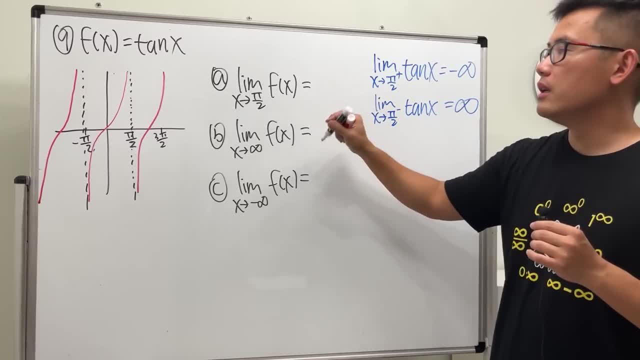 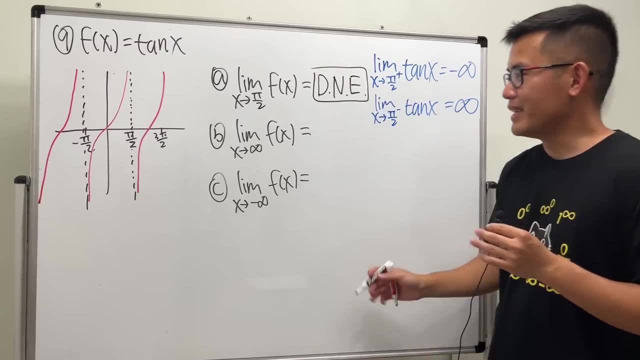 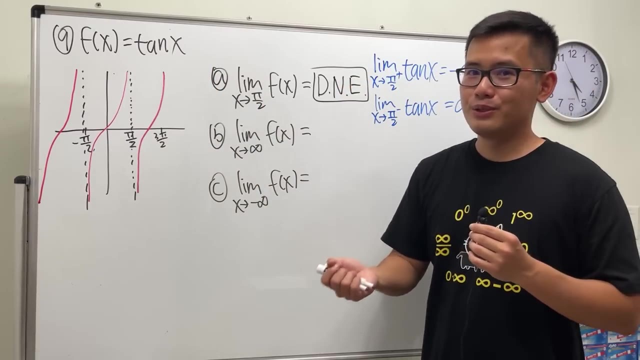 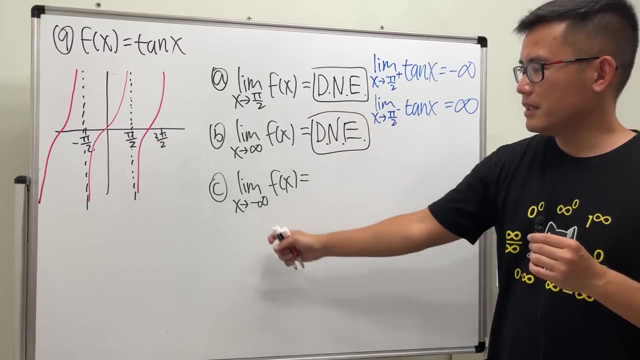 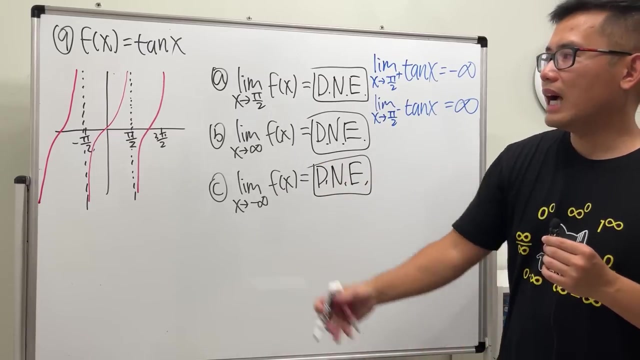 and only one minus can be. the y value does not approach to a particular number, ocean number. so this right here, the d and e. i prefer dots. similarly, x approaching negative infinity, when you have the picture in mind or just draw it down right in front of you. the limit equations: 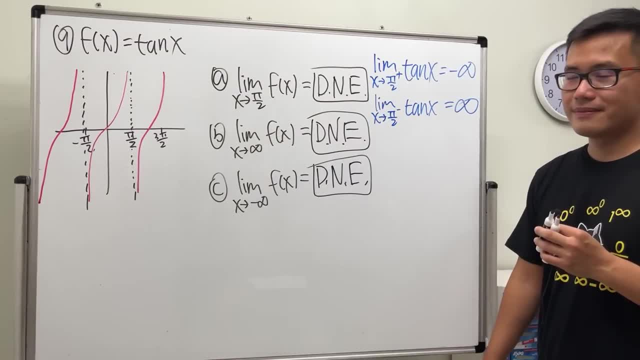 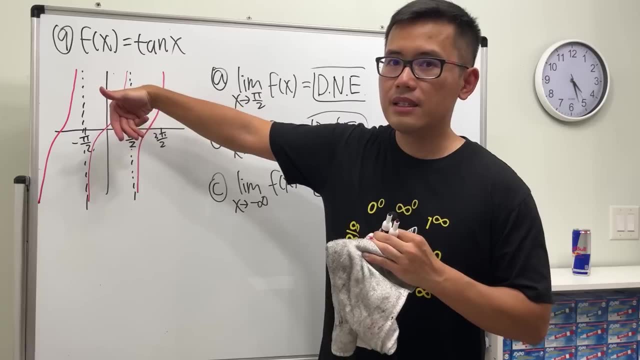 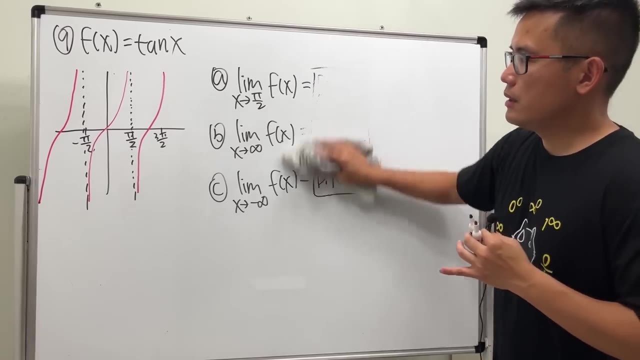 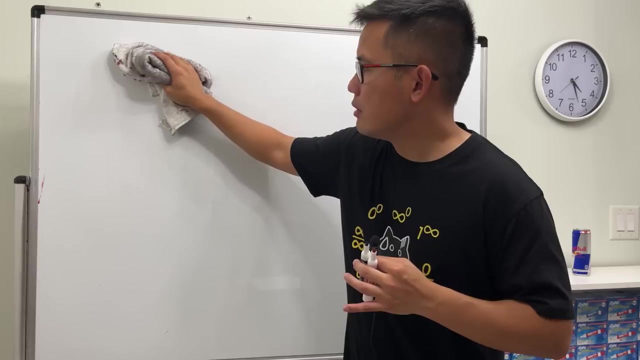 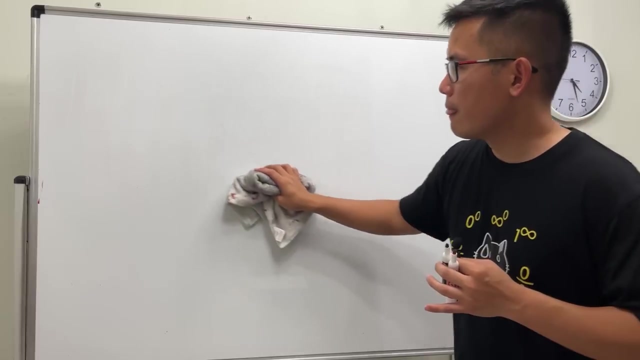 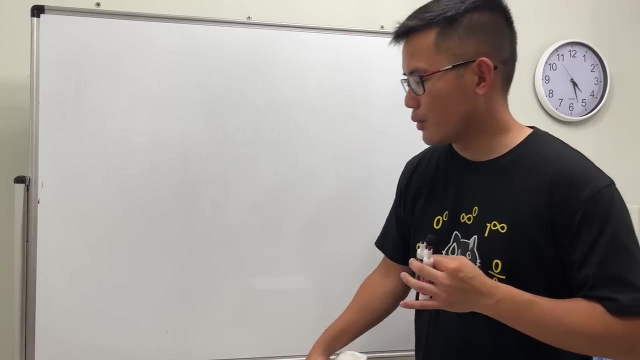 are so much easier, isn't it cool? now we are going to turn this just the middle portion and reflect it about. the line y is equal to x and we get the inverse. so did i graph my original tangent wrong? no, i didn't wait. hold on. 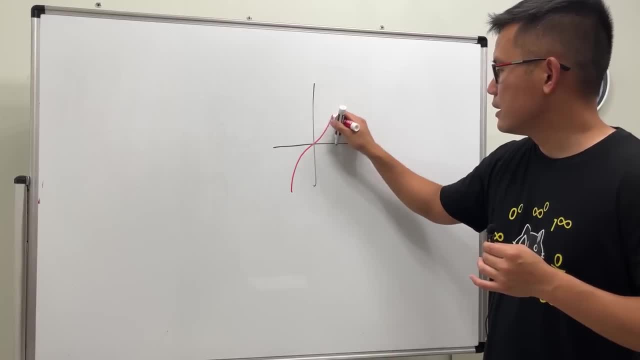 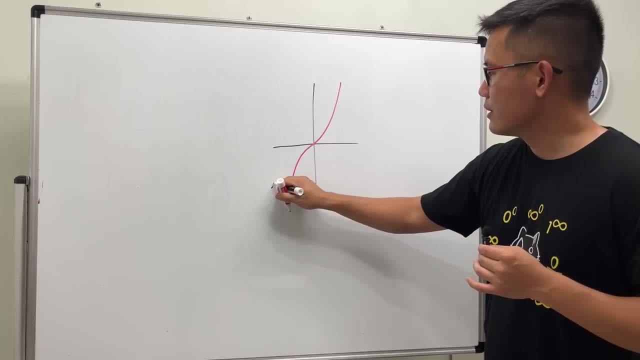 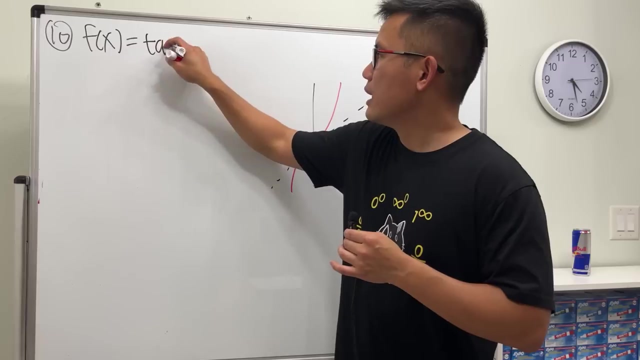 so it was like this: and then i'm going to do a reflection. alright, i'm going to do a reflection, alright. so, anyway, let me do number 10 right here. f of x equals inverse tangent of x. so this was the original tangent and we just 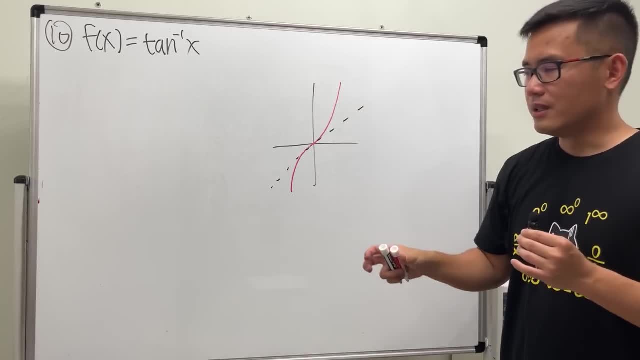 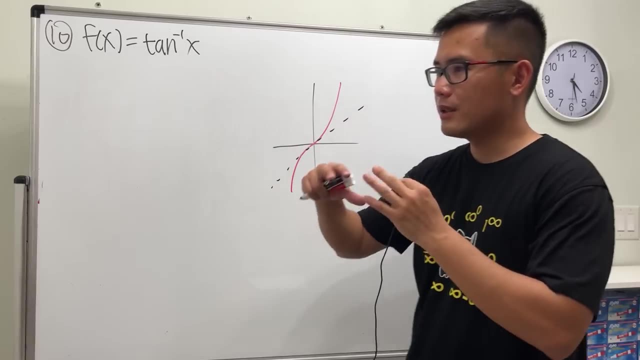 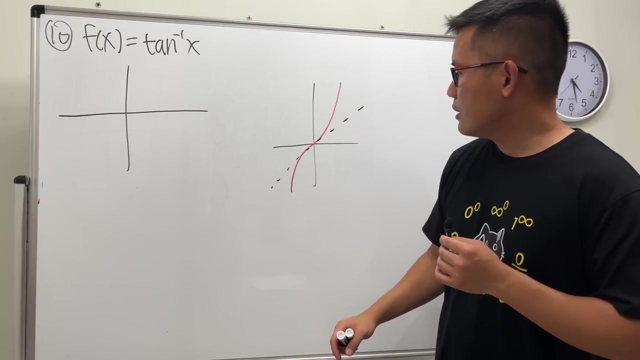 looked at the middle, the first one, because if you do the reflection on everything, then the result is not going to be a function anymore. so just rotate this, flip this, reflect this. so inverse tangent, yeah, uh, um, we are going to get a picture like this: 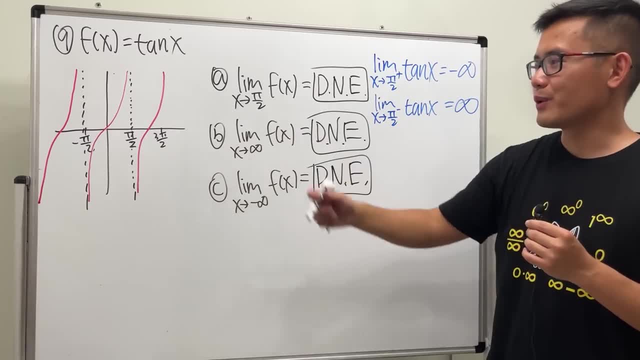 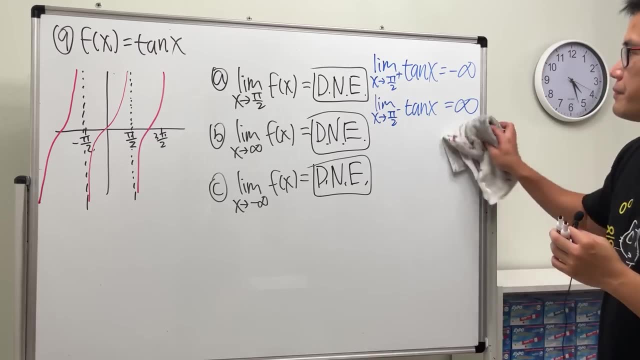 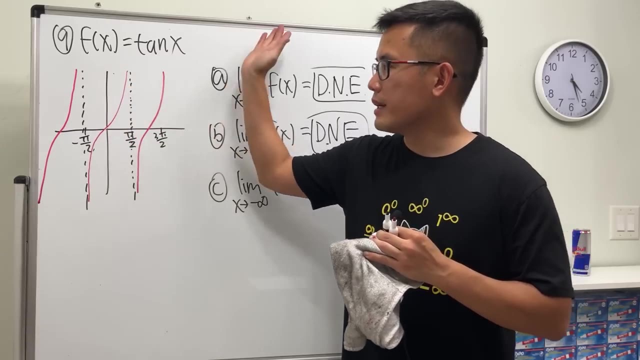 when you have the picture in mind or just right, draw it down right in front of you. the limit questions are so much easier, isn't it cool? now we are going to turn this just the middle portion and reflect it about the line: y is equal to x and we get the inverse right. so 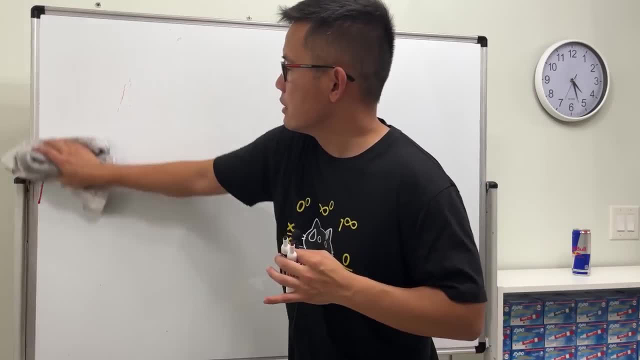 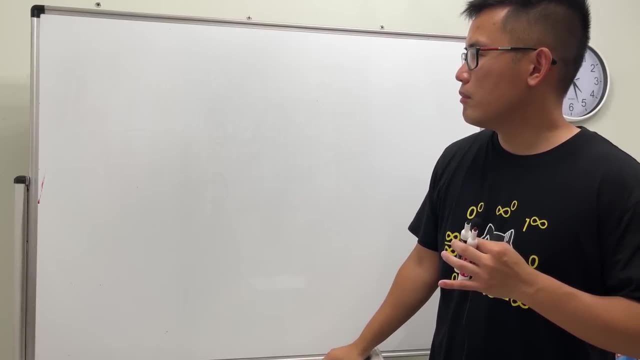 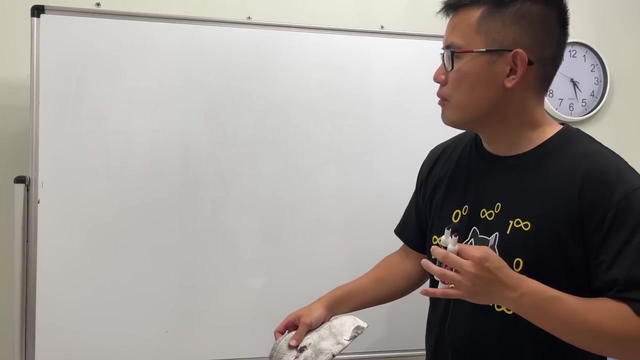 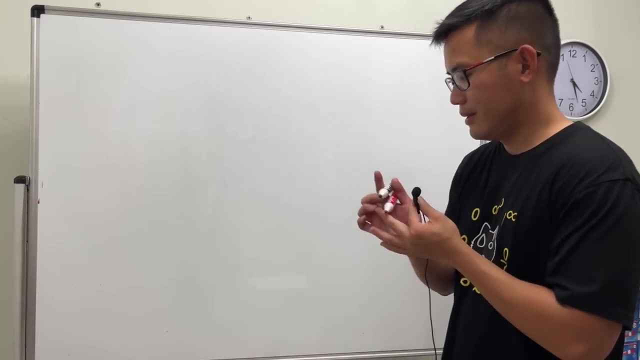 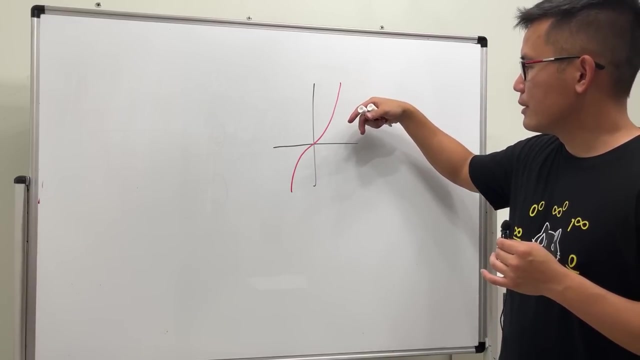 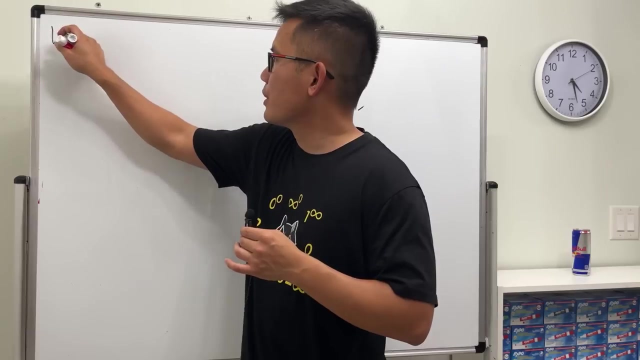 yeah, d, i graphed my inverse, my original tangent, wrong. no, i didn't tangent wait, hold on. so it was like this: and then i'm going to do a reflection. all right, i'm going to do a reflection. so anyway, let me do number 10 right here. f of x equals: 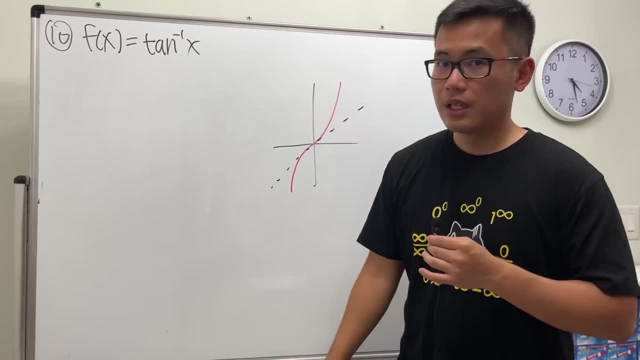 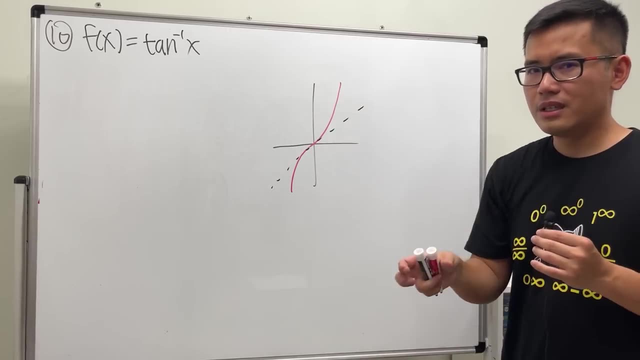 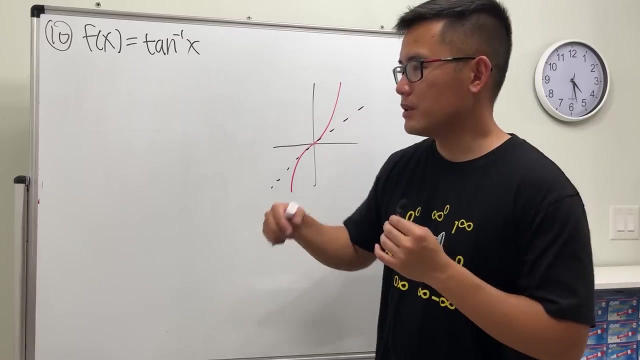 inverse tangent of x. so this was the of x, so this was the original tension and we just, uh, we just look at the middle, like the the first one, because if you do the reflection on everything, then the result is not going to be a function anymore. so just rotate this, not flip this. reflect this, so inverse tangent. 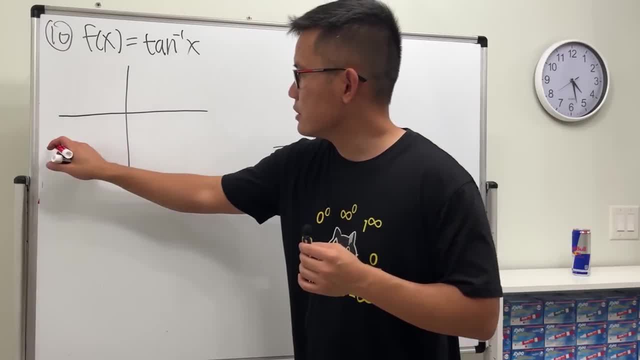 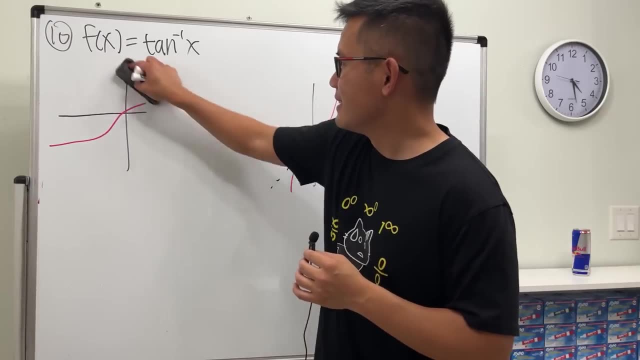 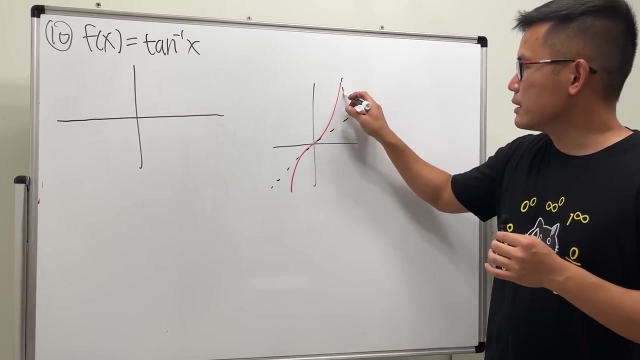 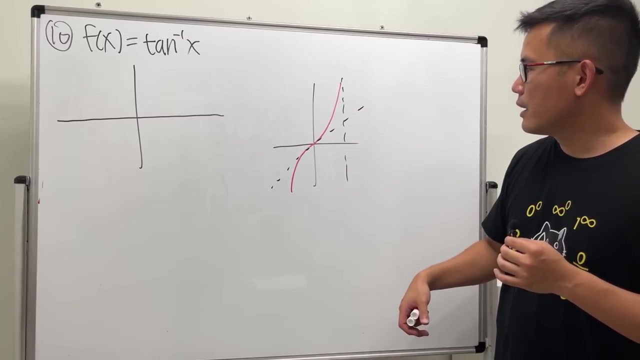 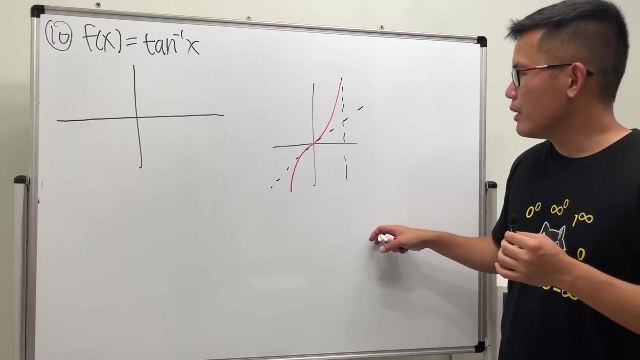 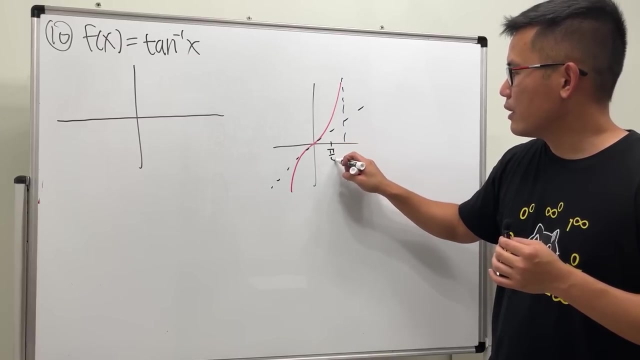 yeah, um, we are going to get a picture like this: ah, let me do it again. all right, this was positive, power over two, right, but if we reflect it, this is going to give us negative pi over two. okay, so we have pi over four, one, and then we will have one pi over four. so yeah, 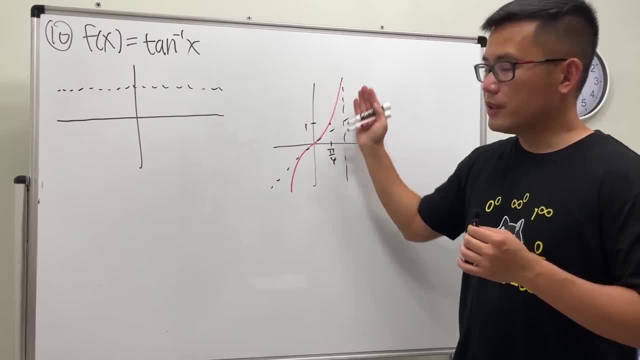 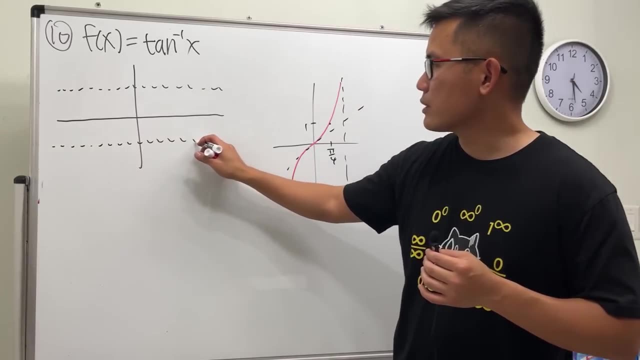 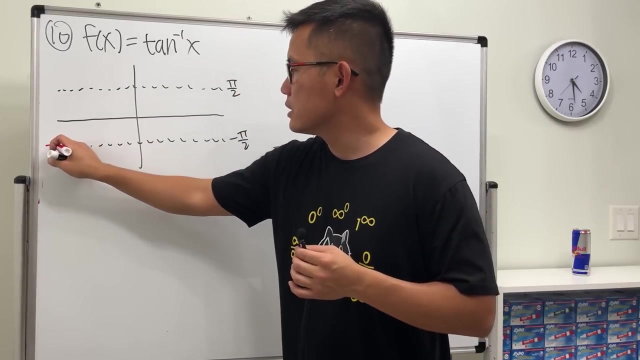 yeah, yeah, what am i talking about anyway? so, if we reflect it, this vertical as though will become horizontal as though, and then this vertical as though, which is at negative pi over two, will be another horizontal. so this right here is negative pi over two and this is pi over two, and 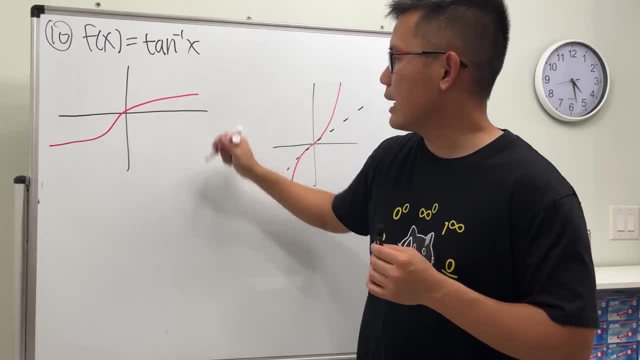 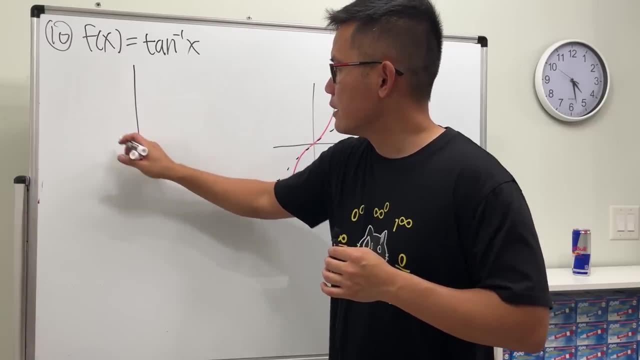 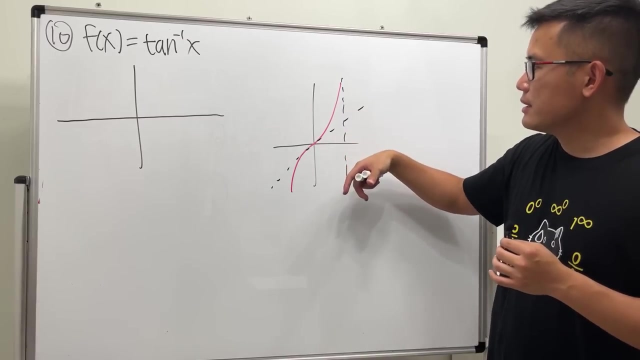 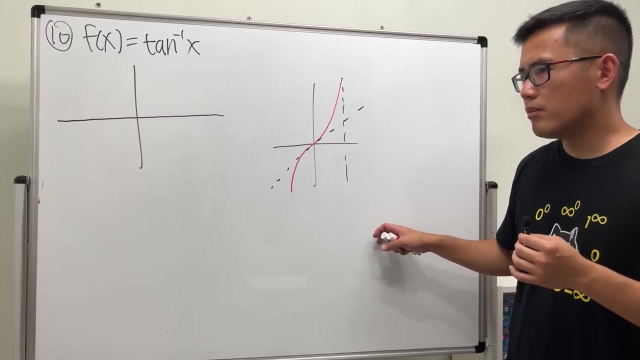 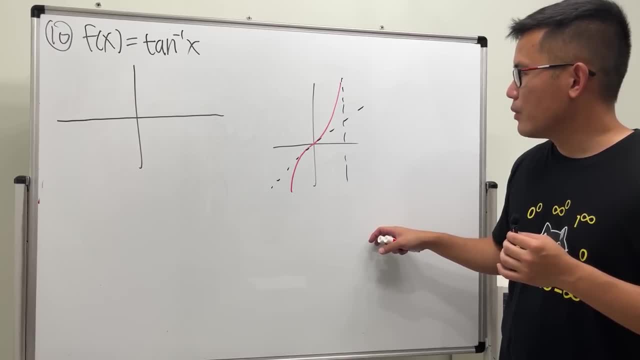 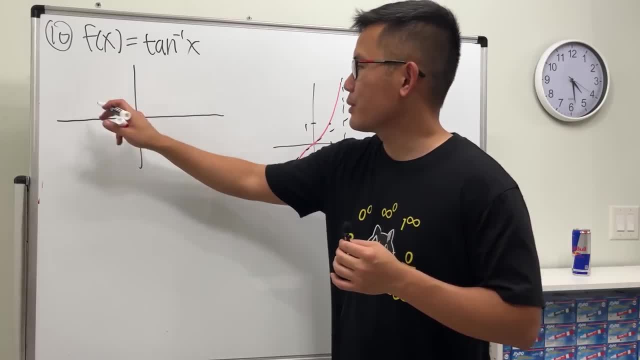 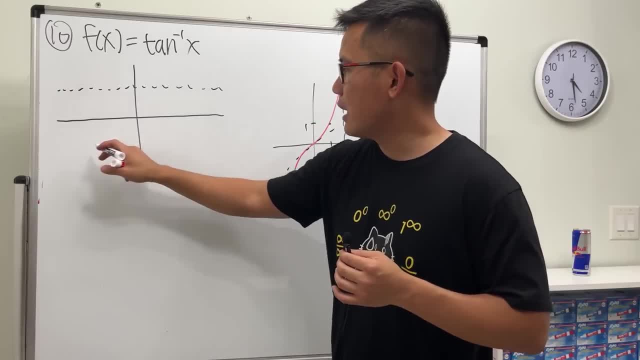 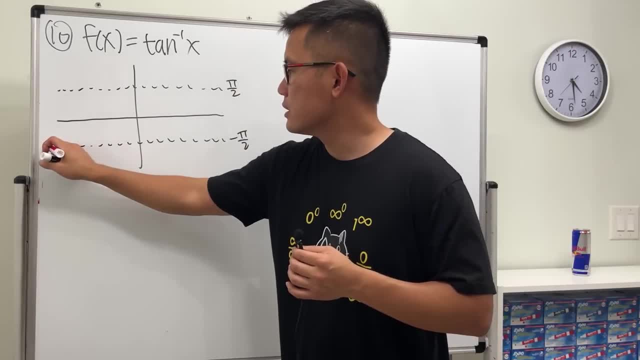 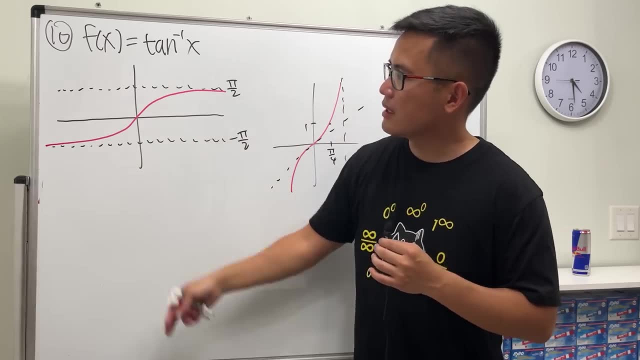 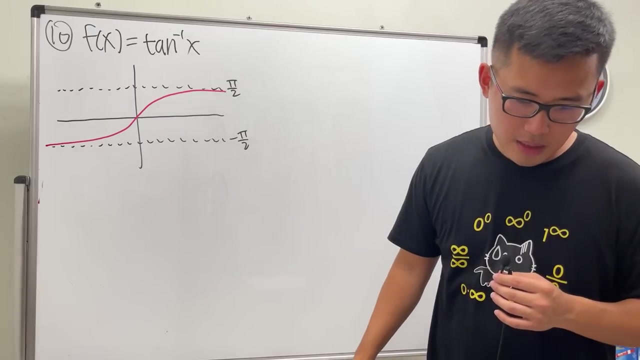 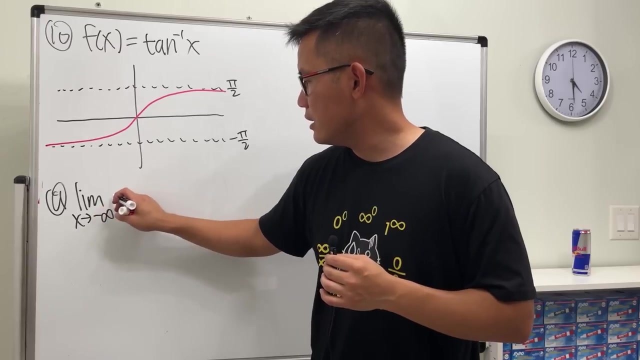 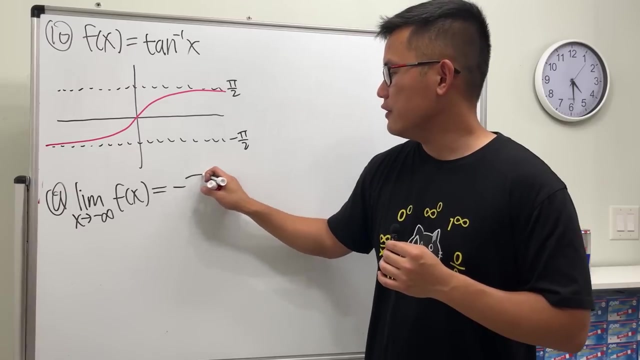 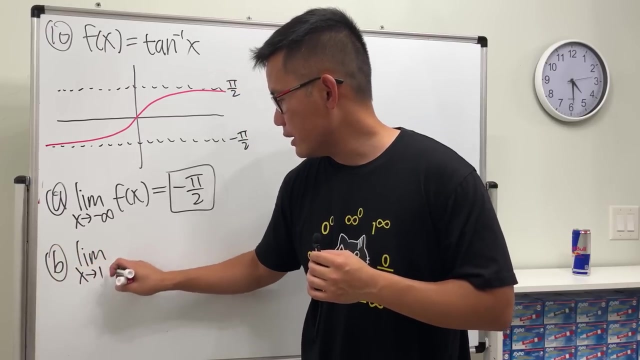 pi over two and the curve looks like this: okay, so it has that two boundary, but yeah, that's horizontal isotopes anyway. and this is number 10. and here we go: a limit X approaching negative infinity of our function. if it goes to negative infinity, we get negative pi over two. be limit X approaching one F of 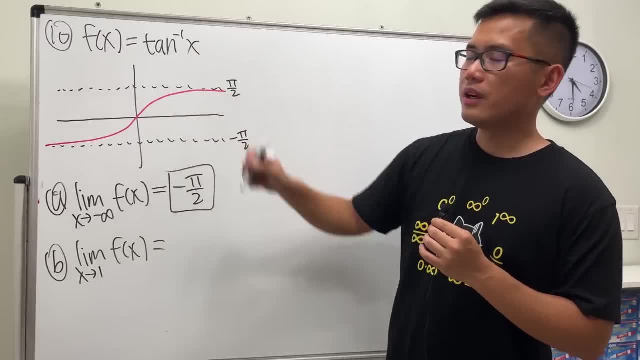 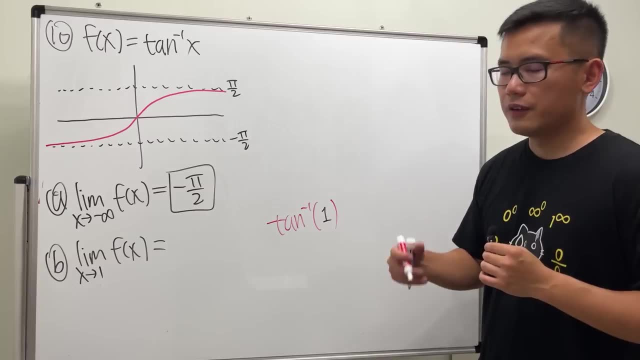 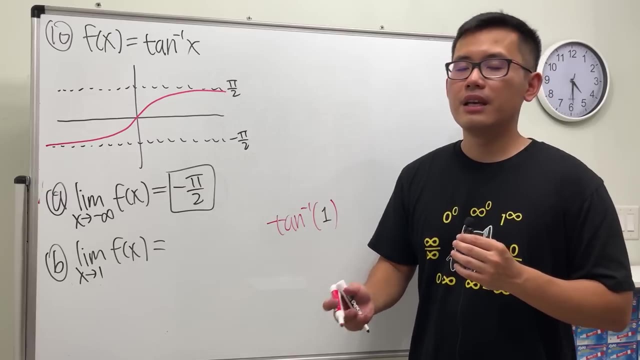 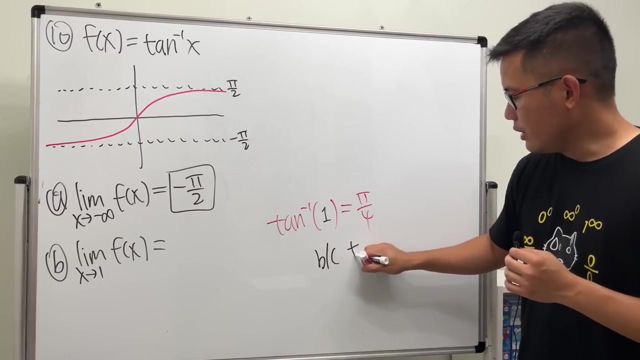 X. we can just simply put one in here, inverse tangent of one. how do we do this? we will have to ask ourselves: tangent right, the original tangent of what angle will give us one? look at the first answer and the answer for that is pi over four. so this right here is pi over four. and again the reasons: because regular. 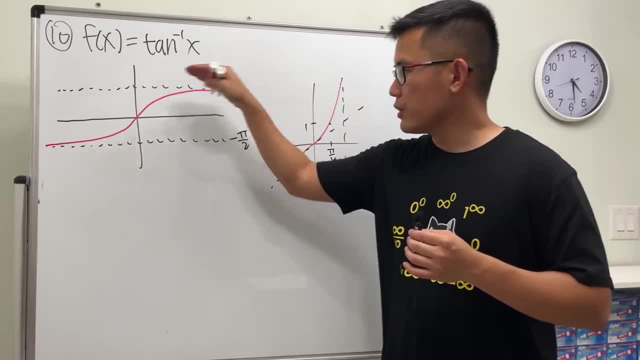 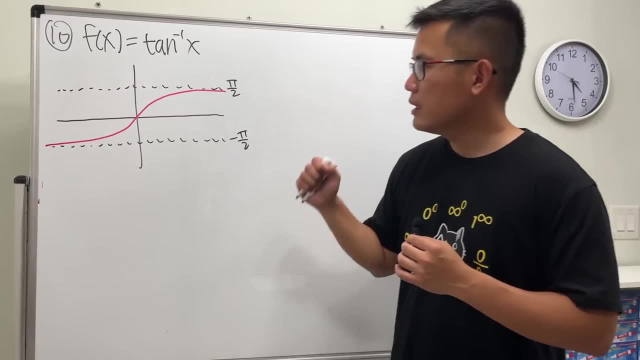 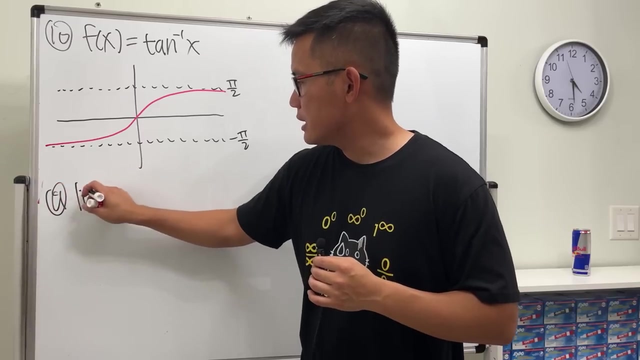 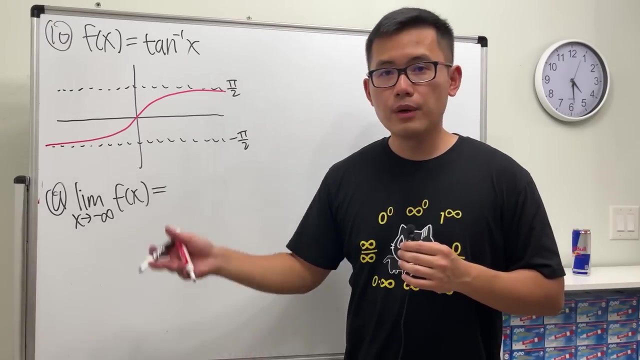 the curve looks like this: okay, so it has that two boundary, but yeah, that's horizontal isotopes anyway. this is number 10. and uh, here we go. a limit x approaching negative infinity of our function. if it goes to negative infinity we get negative pi over two b. 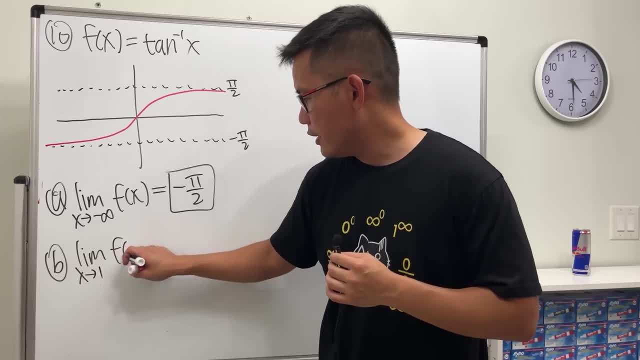 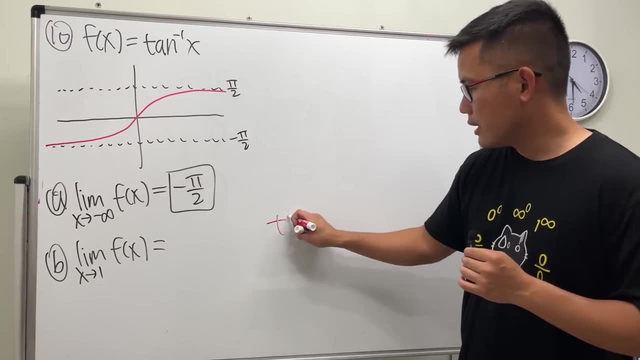 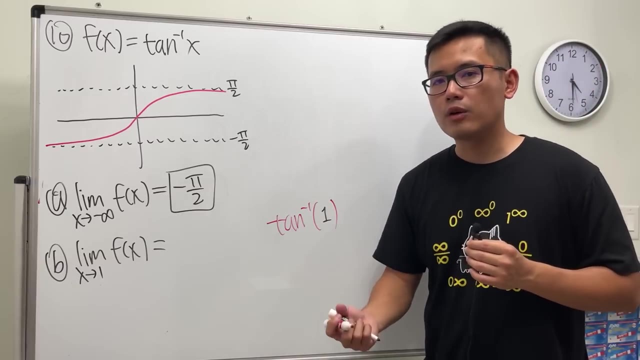 limit x approaching one f of x, we can just simply put one in here, inverse tangent of one. how do we do this? we will have to ask ourselves: tangent right? the original tangent of what angle will give us one. look at the first answer. and the n set of a is pi over 4.. so this right here. 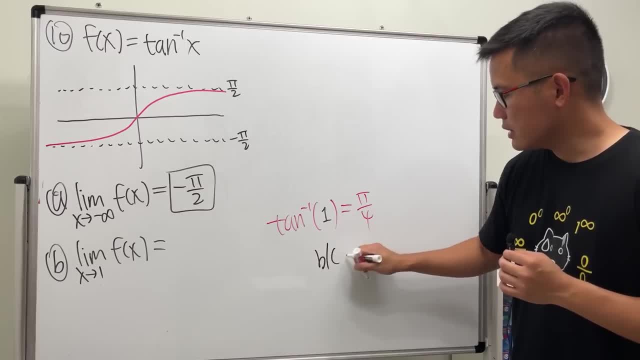 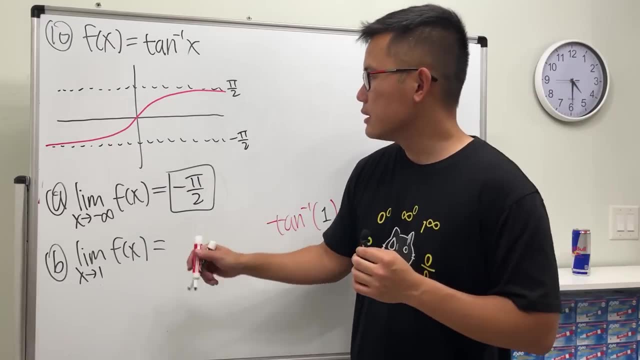 is pi over 4.. and again, the reason is because regular tangent of four one is 8 and negative pi- am i saying it is magic of pi over four gives us one And it's nice and continuous. so that's why when x is approaching one, 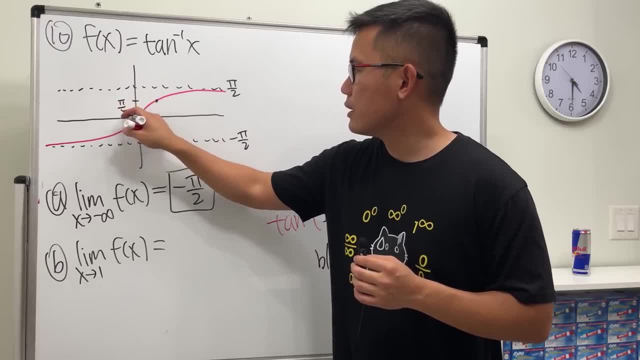 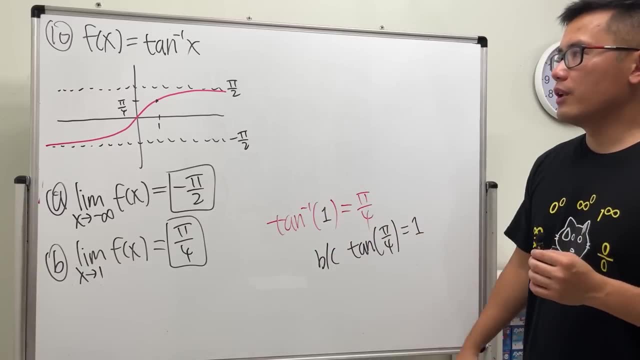 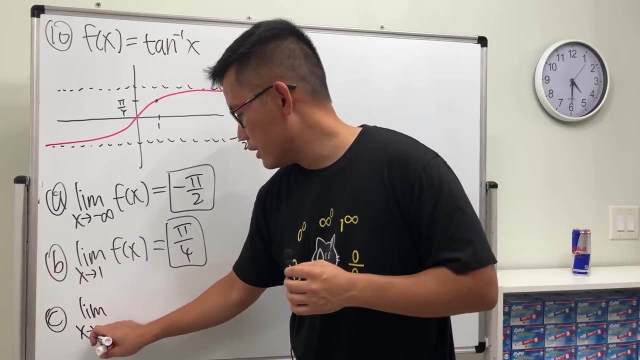 this y value is pi over four. So this is one of the values that you should remember. It's going to happen a lot. Inverse tension is one of the very common function that you have to deal with in your calculus class, not just for limits but also later on for the derivative. 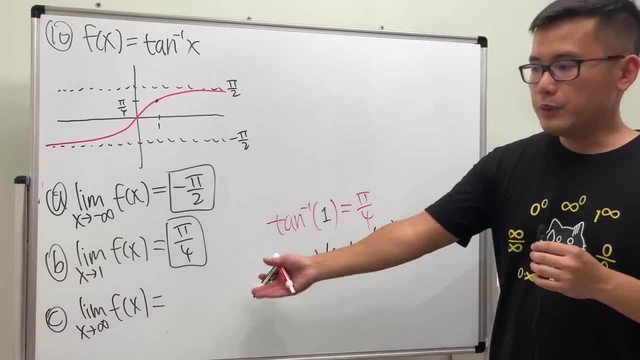 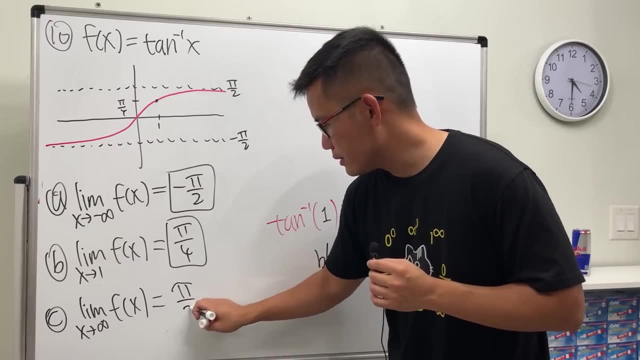 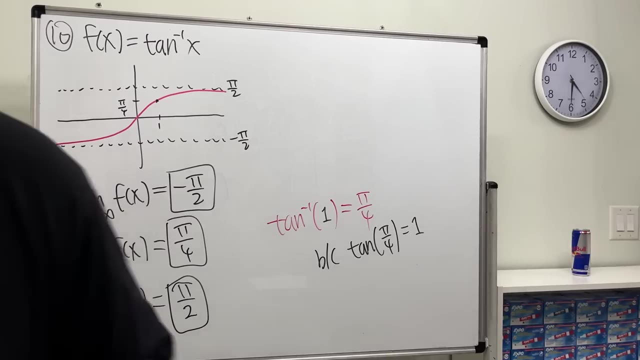 and also the integral. Anyway, last one, The limit as x approaching positive infinity, we get positive pi over two. Ah, so much better when we have a graph in front of us. right, Certainly 10 questions. let me just check. 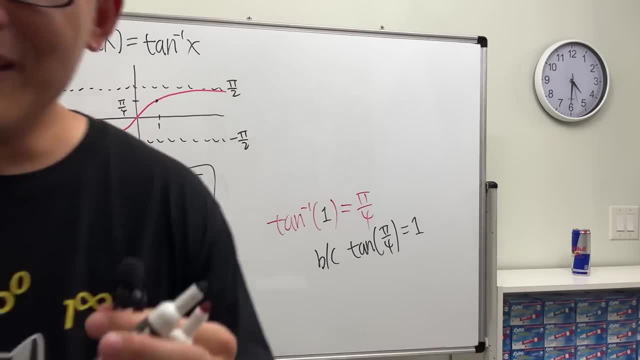 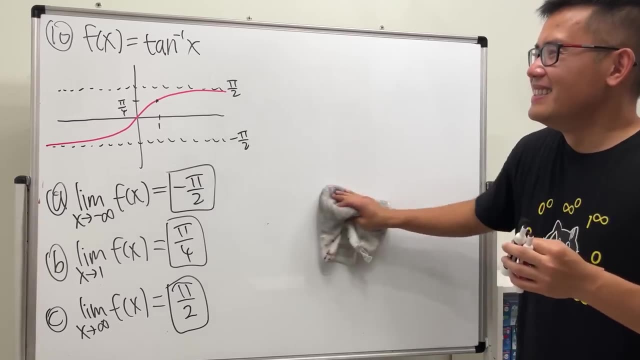 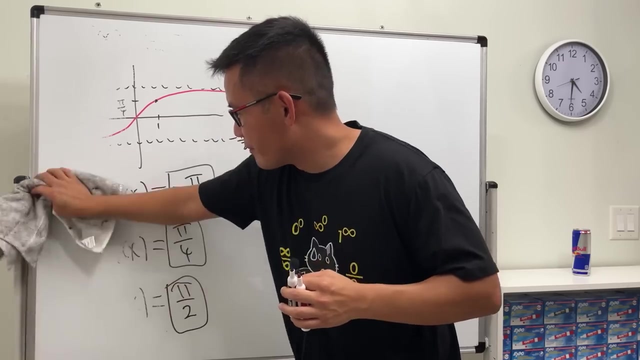 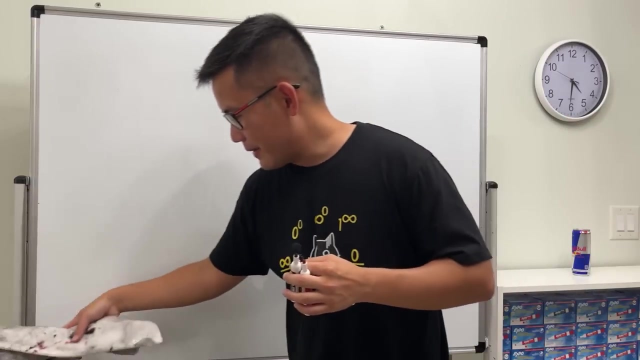 Good, Wait, how long did I take? Wow, 56 minutes for 10 questions. are you serious? Wow, I thought it was just like 30 minutes. Oh, my goodness. Okay, so that's the first category. We determined the limits from a graph. 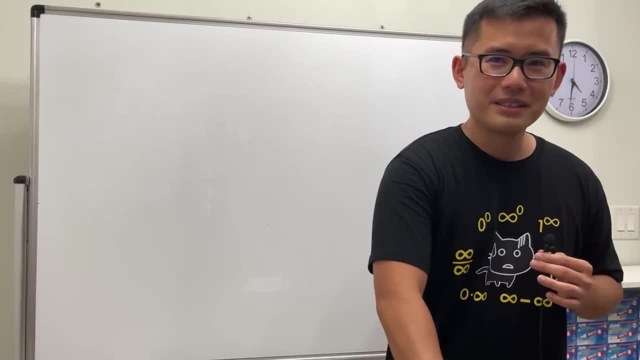 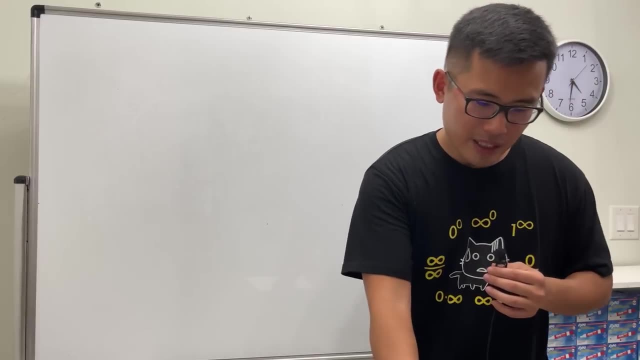 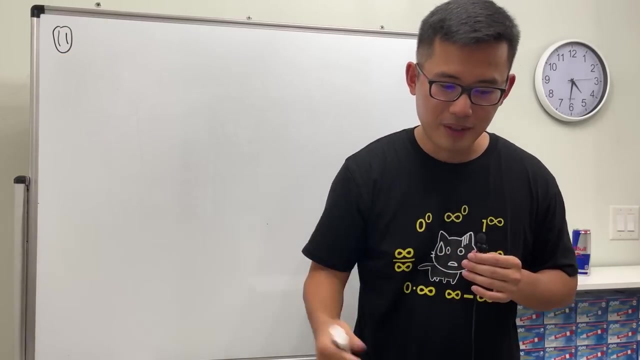 And the second category is still kind of similar. Depends on how you want to do it. We will see how to find the limit from piecewise functions. Okay, so number 11. At least this time that we are just doing one question per question. 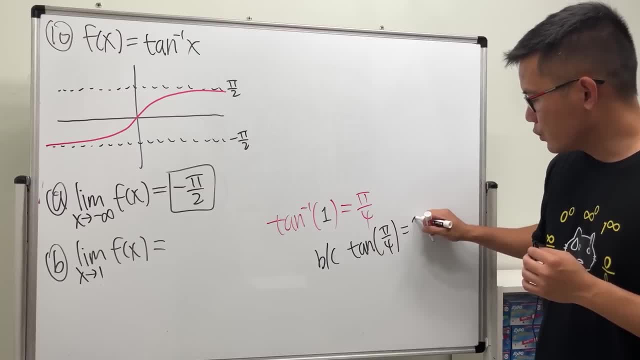 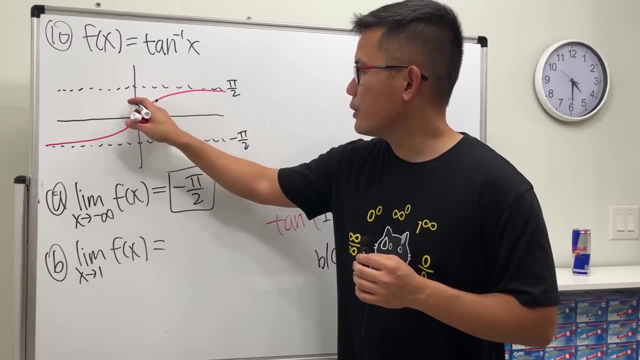 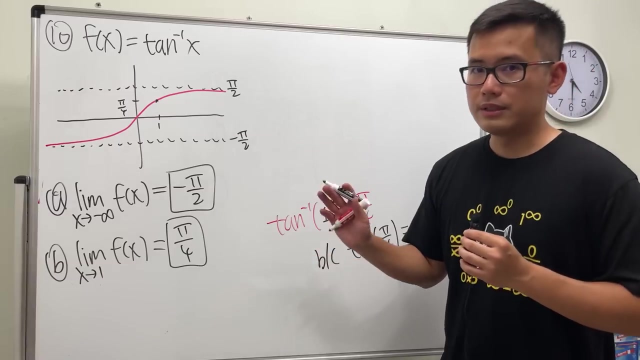 tangent of pi over four gives us one and it's nice and continuous. so that's why, when X is approaching one, this Y value is pi over four. so this is one of the values that you should remember. it's going to happen a lot. inverse tension is one of the very common function that you have to deal. 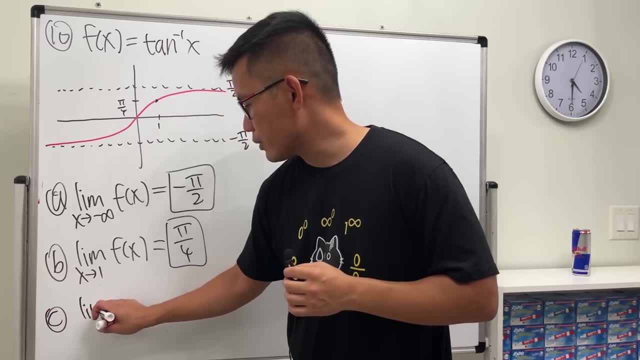 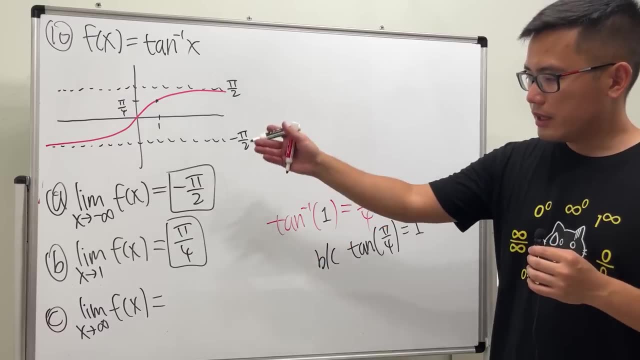 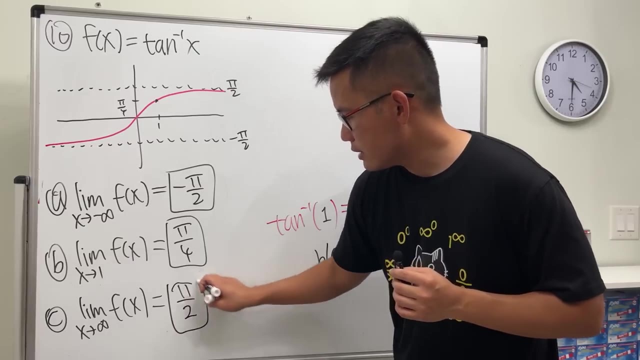 with in your calculus class, not just for, but also later on for the derivative and also the integral. anyway, last one: the limit. as X approaching positive infinity, we get positive pi over 2. ah, so much better when we have a graph in front of us. right, certainly. ten questions, let me. 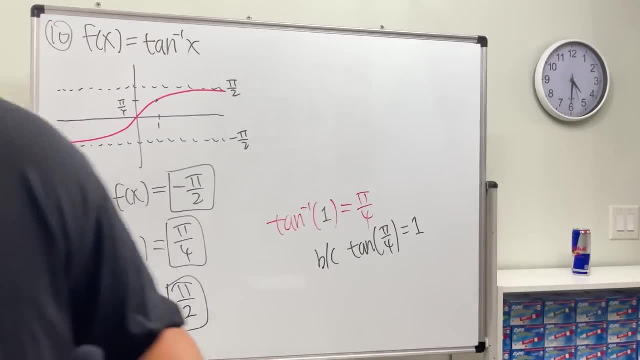 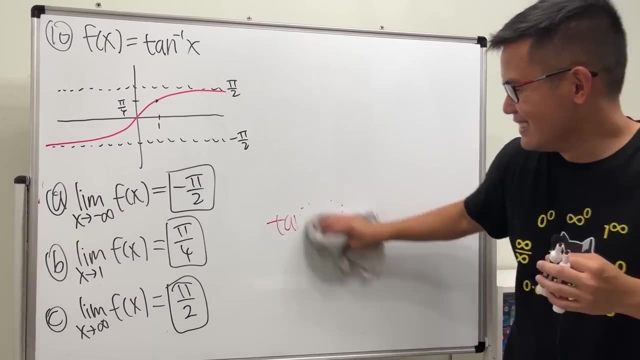 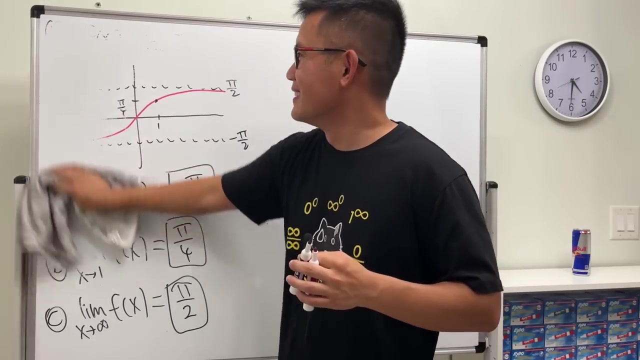 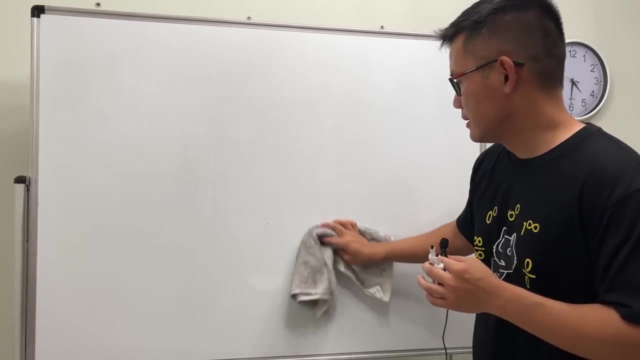 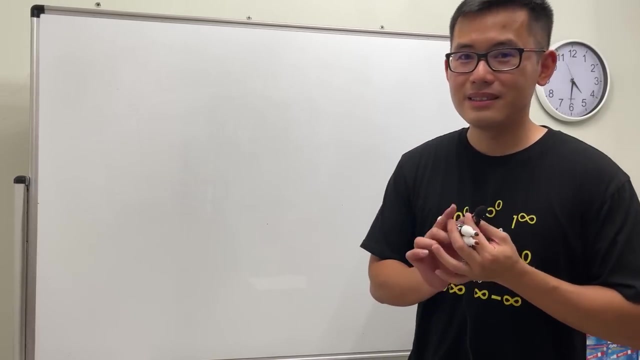 just check. good wait, how long did I take? Wow, 56 minutes for ten questions. are you serious? Wow, I thought it was just as 30 minutes, oh my goodness. okay, so that's the first category with determine the limits from a graph, and the second category is still kind of similar. 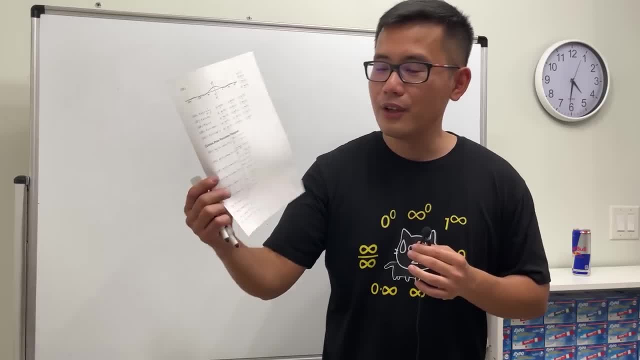 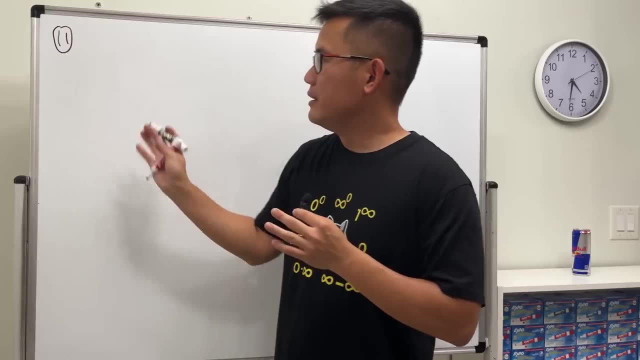 depends on the second category, and the second category is still kind of similar. how you want to do it, we will see how to find the limit from piecewise functions, okay, so number 11 at this this time that we are just doing one question per per question earlier was like three questions per question anyway. 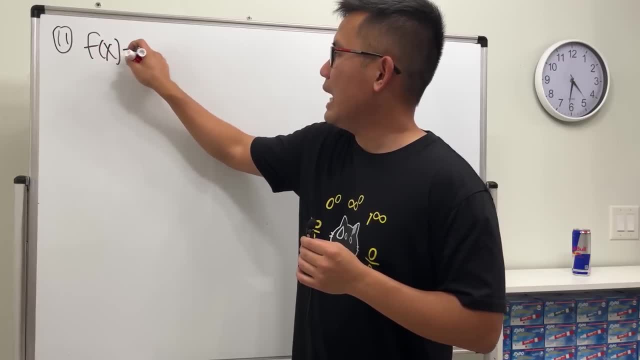 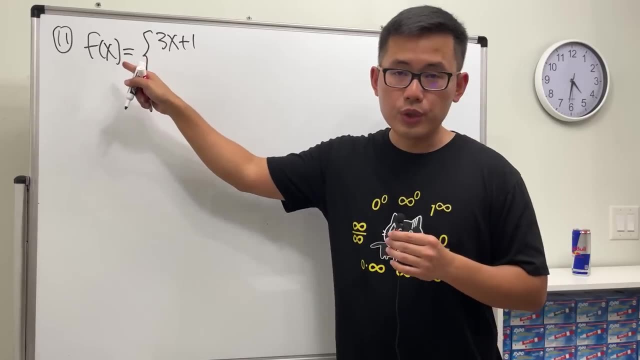 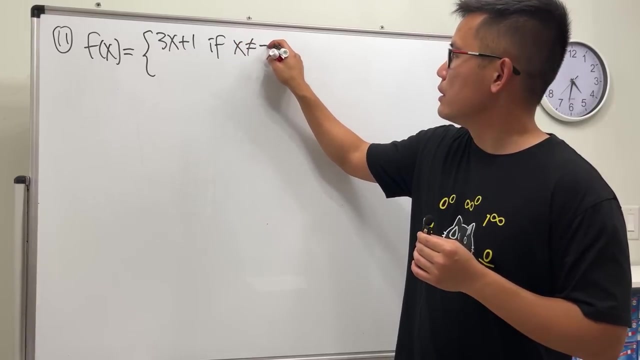 i'm going to give you guys the function here, right here. so we have our function. f of x is the piecewise function. you just have to pay attention to the conditions. so here we do 3x plus 1. this is when x is not equal to negative 2. but when x is equal to negative 2, we get 2. so 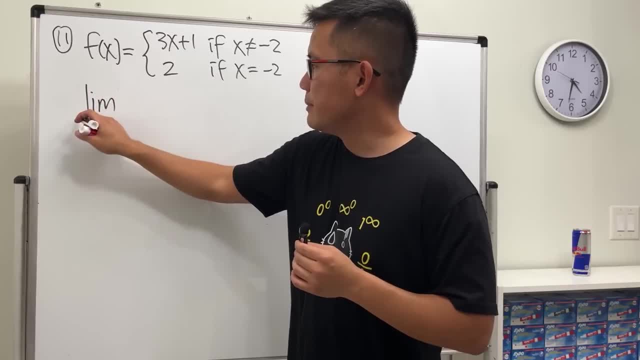 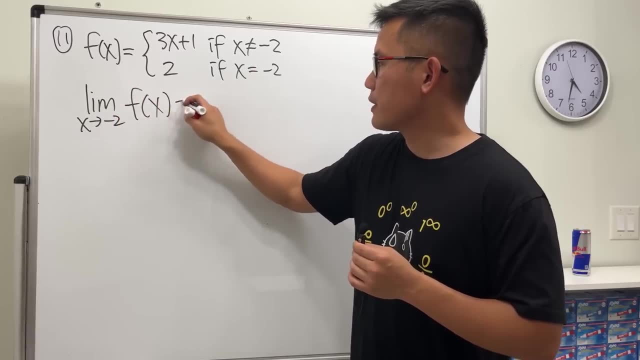 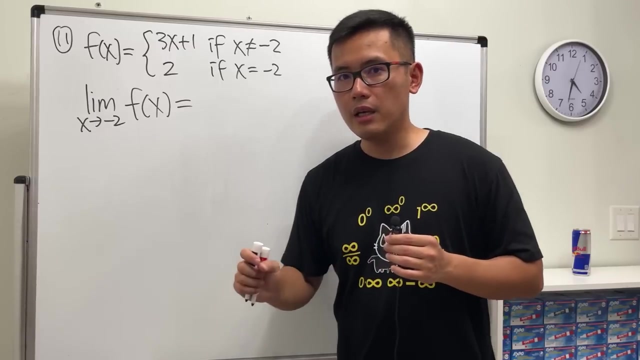 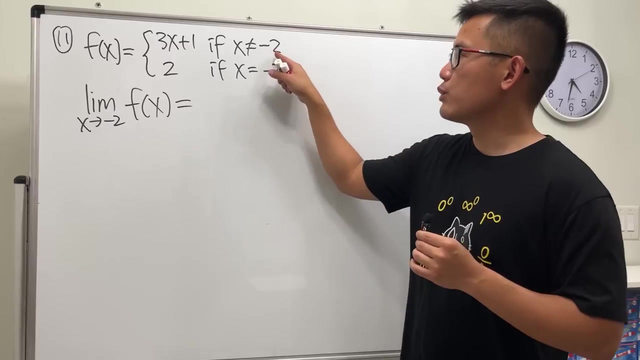 so just like this, and our goal is to find the limit as x approaching negative 2. of course, that will be the interesting number of the function. so here's the deal. when we're talking about the limit as x approaching negative 2, we do not care about. x is at exactly negative 2, so we don't care about this, we just have to worry. 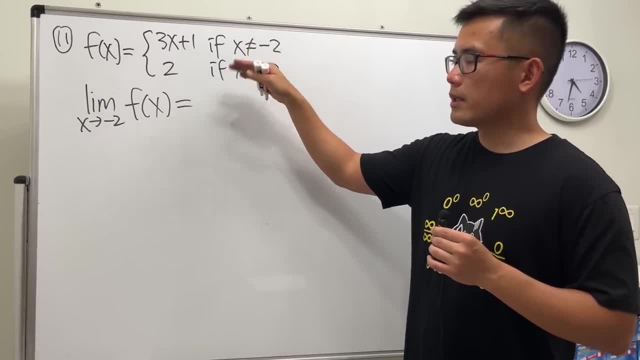 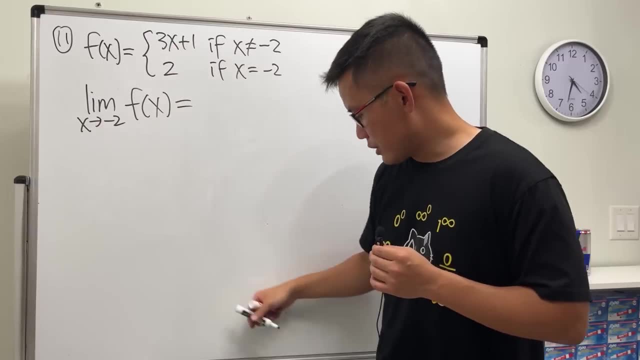 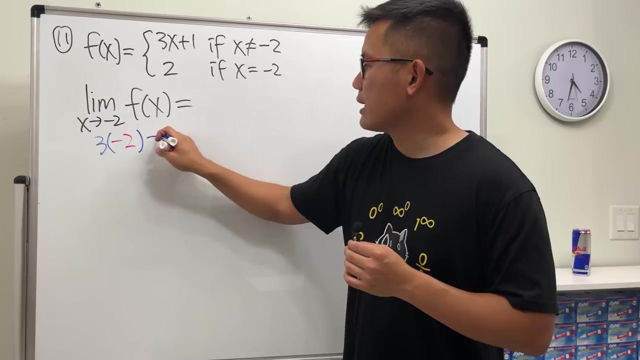 about this and, uh, you don't have to worry about the left and right, because left and right is just this anyway. so we can just put negative 2 into here. so let's just do a computation real quick. we will just get three times negative 2 plus 1. work that out, we get negative 5. 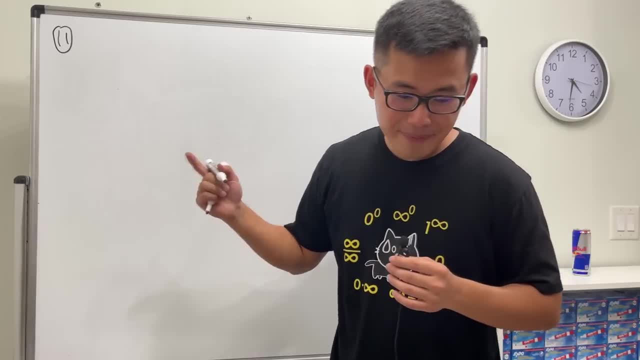 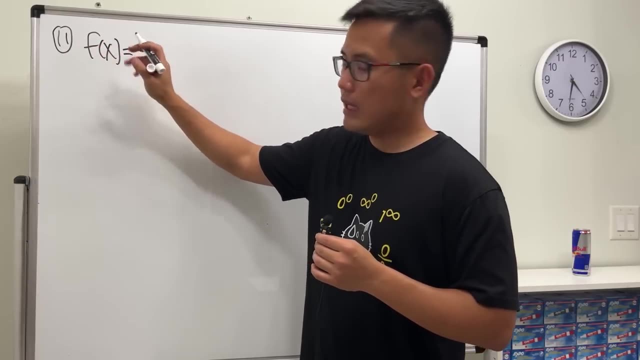 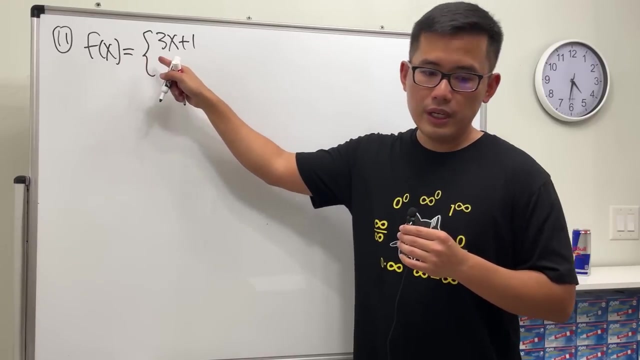 Earlier was like three questions per question. Anyway, I'm going to give you guys the function here, right here. So we have our function f of x. it's a piecewise function, You just have to pay attention to the conditions. So here we do, three x plus one. 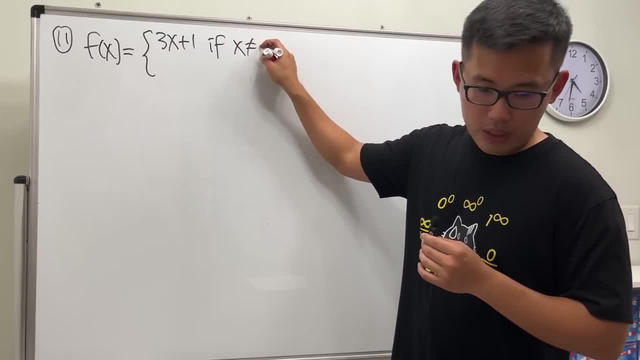 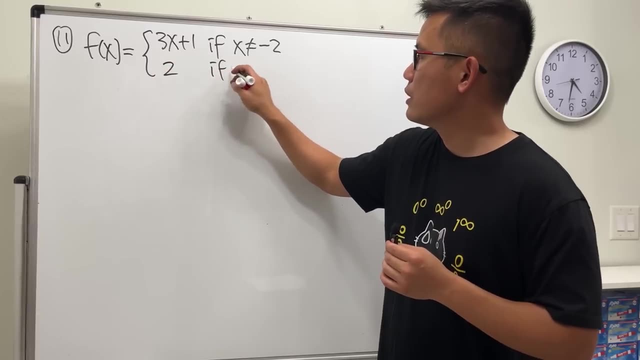 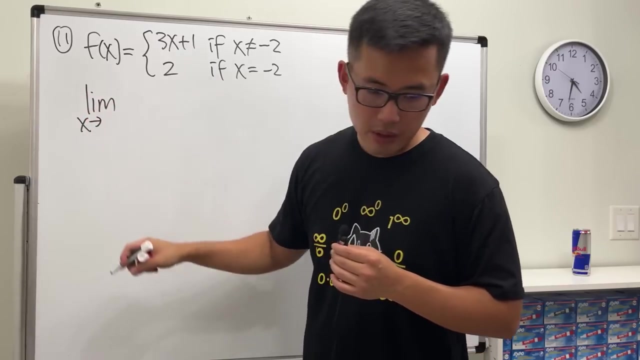 This is when x is not equal to negative two. But when x is equal to negative two, this is when x is not equal to negative two. So if x is equal to negative two, we get two. So just like this. And our goal is to find the limit as x approaching negative two. 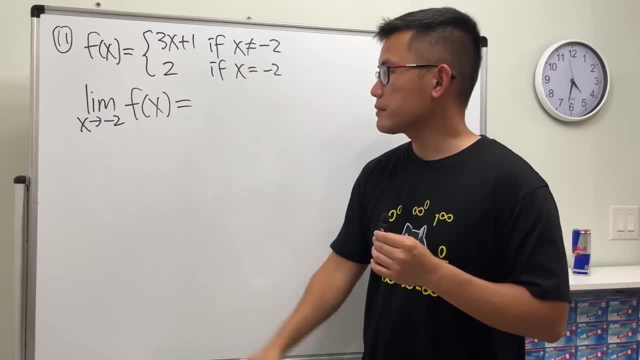 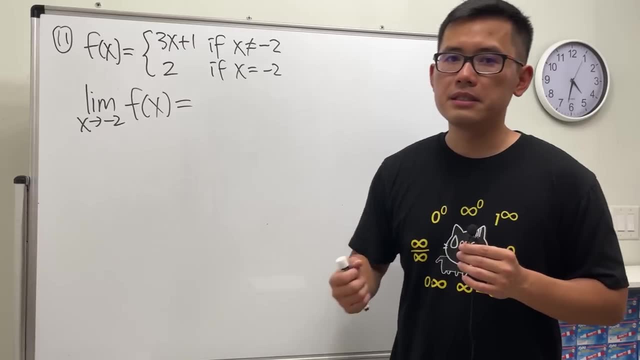 Of course, that will be the interesting number of the function. So here's the deal. When we're talking about a limit as x approaching negative two, we do not care about. x is at exactly negative two, So we don't care about this. 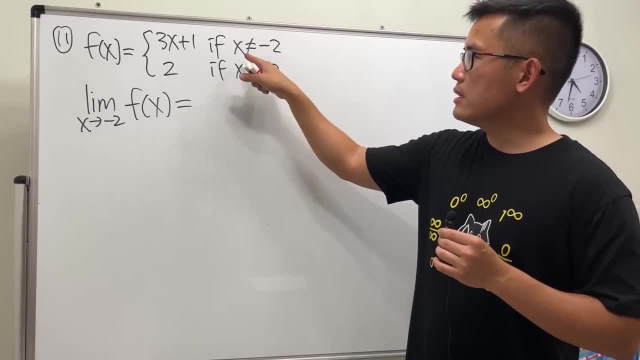 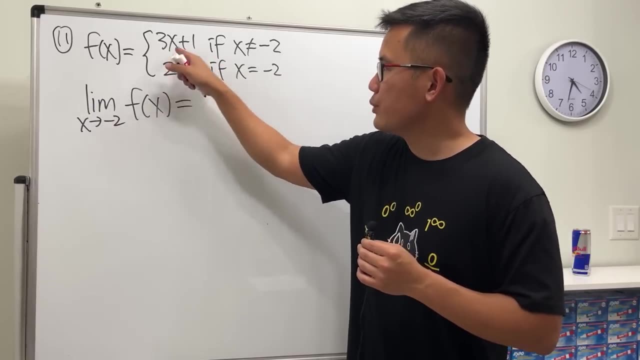 Okay, We just have to worry about this, And you don't have to worry about the left and right, because left and right is just this anyway. So we can just put negative two into here. So let's just do a computation real quick. 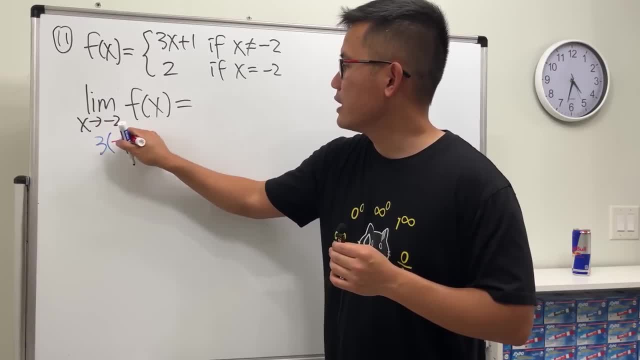 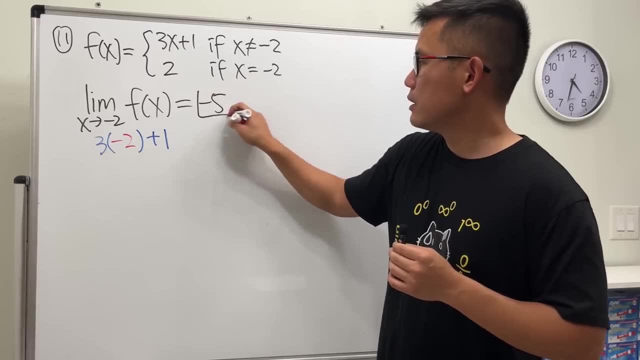 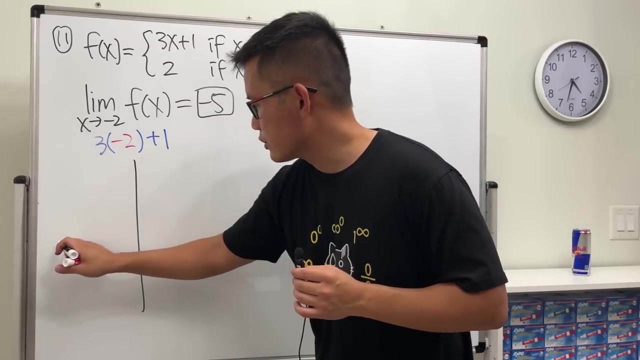 We will just get three times negative, two plus one. Work that out, we get negative five And that's it. All right, Seriously, that's it. I will give you guys a picture, real quick, Real quick, to illustrate why this is the case. 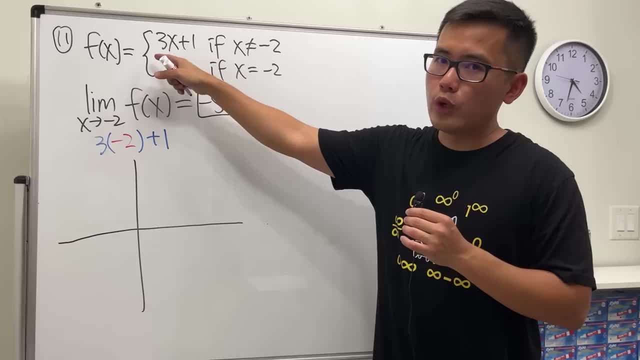 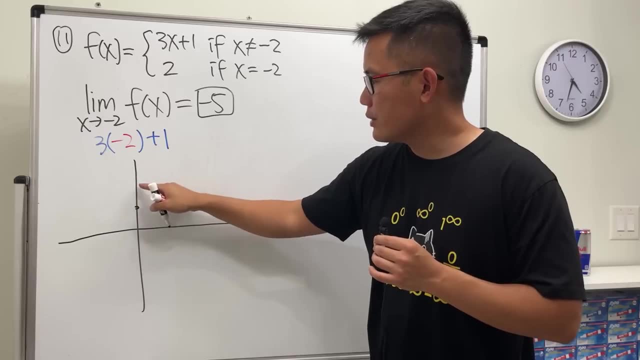 Firstly, let's focus on graphing this, which is just the equation of a line: The y intercept is at one And then the slope is three, meaning that we go up three times- one, two, three- and then go to the right one time. 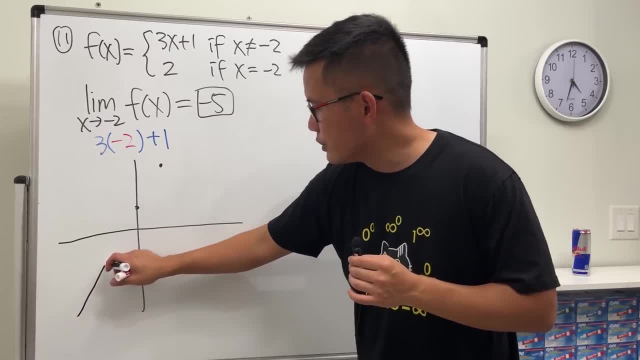 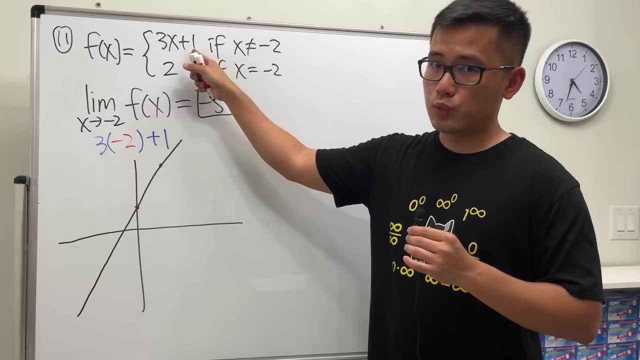 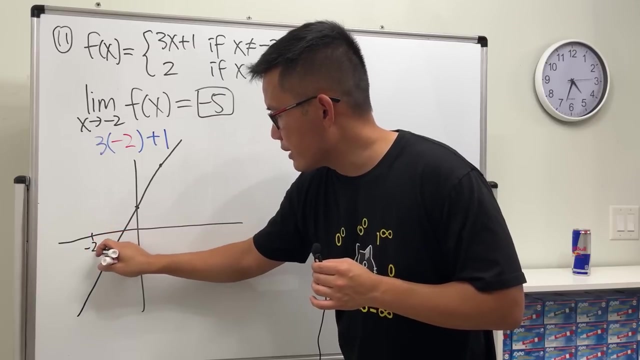 Well, you don't have to be like super precise, You just have to make sure that your picture makes sense. So this is the equation of the line three: x plus one. However, X cannot be equal to negative two. It means that we will have to go to when x is equal to negative two. go to the line and: 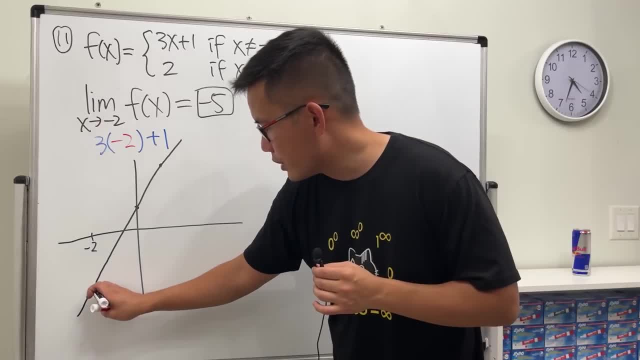 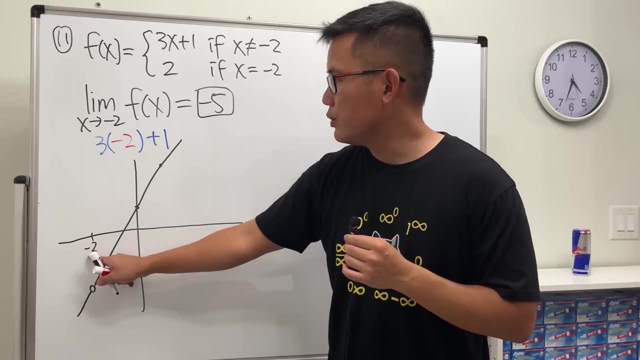 then erase it And then we'll put an open circle here. But now the question is: what's the y value for this open circle To do? so? we put negative two into here, Just pretend that the point was still there, And then we saw that it was negative five. 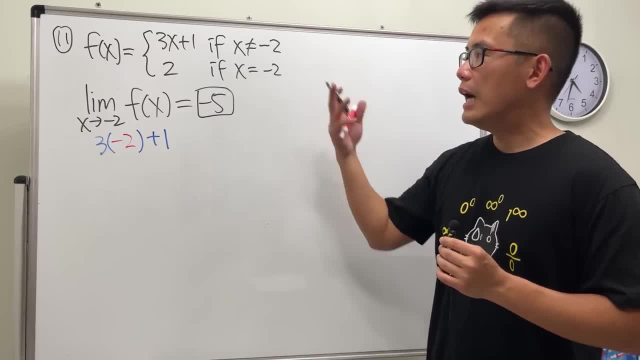 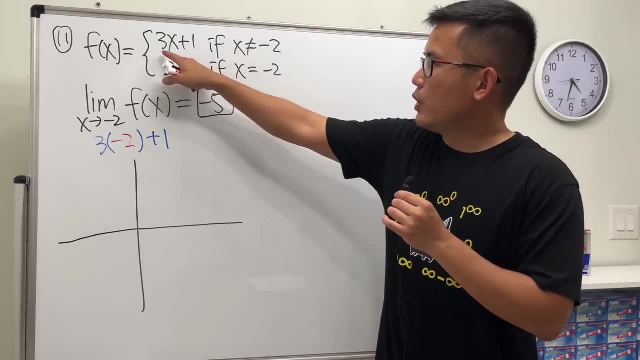 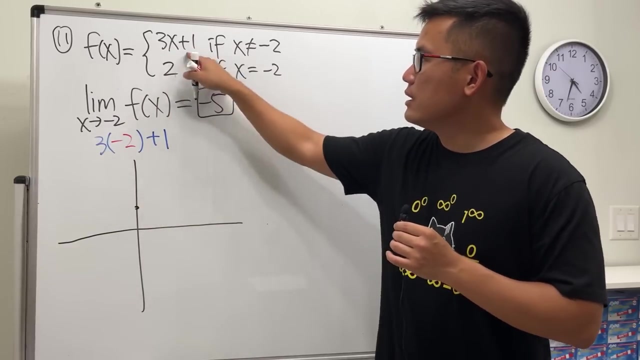 and that's it. all right, seriously, that's it. i will give you just a picture, real quick, to illustrate why this is the case. firstly, let's focus on graphing this, which is just the equation of a line: the y intercept is at 1 and then the slope is 3, meaning that we go up three times- one, two, three- and then go to. 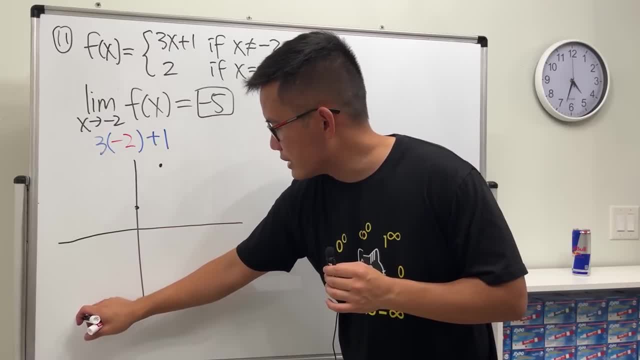 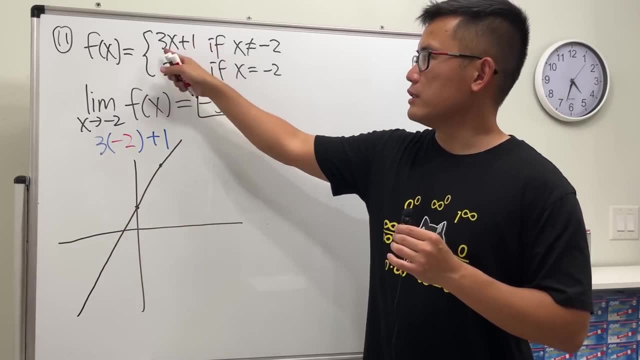 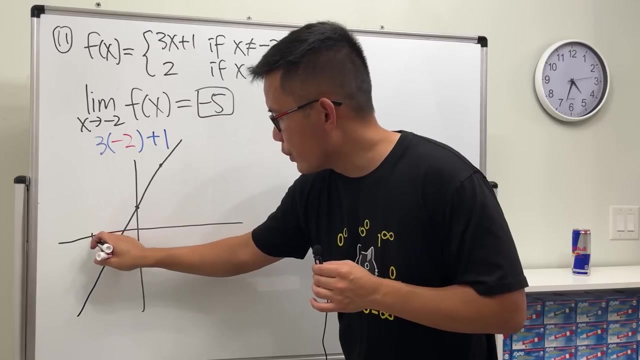 one time. well, you don't have to be like super precise, you just have to make sure that your picture makes sense. so this is the equation of the line 3x plus 1.. however, x cannot be equal to negative 2.. it means that we will have to go to when x is equal to negative 2, go to the line and. 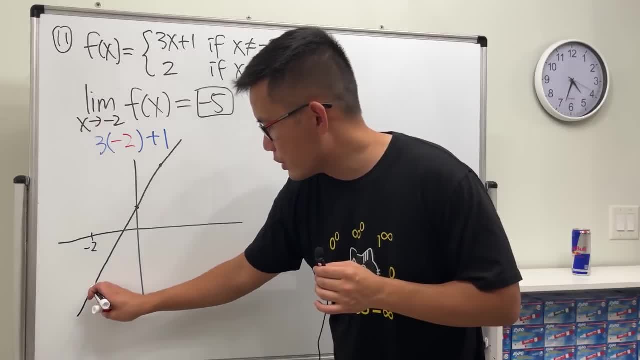 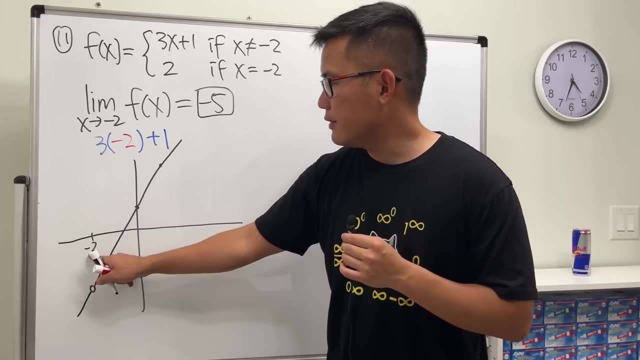 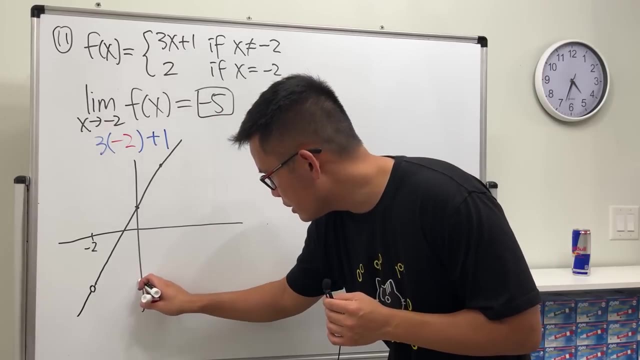 then erase it and then we'll put an open circle here. but now the question is: what's the y value for this open circle to do? so? we put negative 2 into here, just pretend that the point was still there, and then we saw that it was negative 5.. so this right here is negative 5.. however, we still 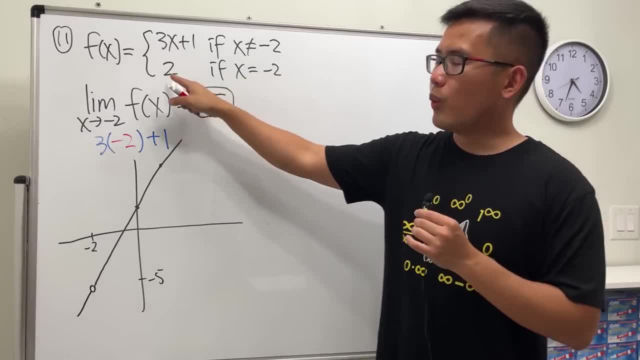 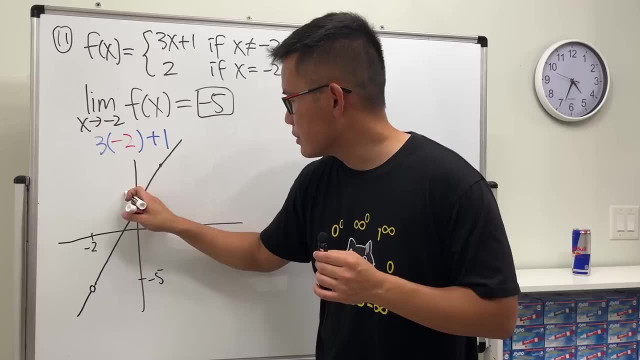 have to grab the second piece. when x is negative 2, the y value is actually at 2.. so when x is negative 2, we actually go up to 2, right here. this is 2, let's say this is 2, and then we have a. 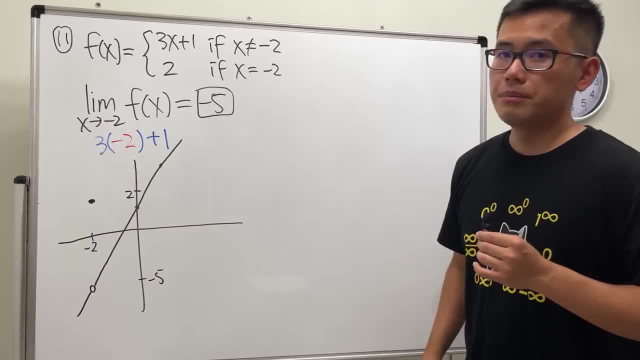 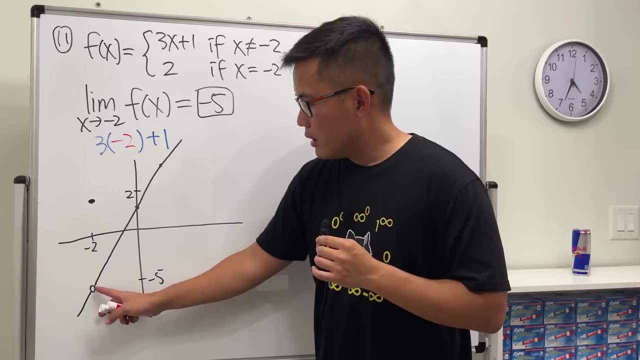 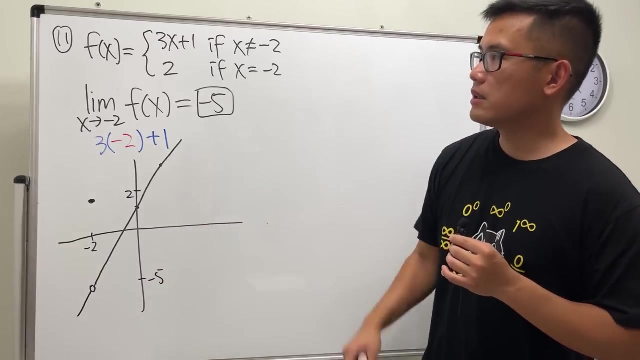 closed circle. so this right here will be the picture for this piecewise function. and now you should be clear that again, just like what we did in the first category, when x is approaching negative 2 from the left and from the right, both of, uh, both of them give us negative 5.. the answer is negative 5.. done, deal, right. so that's number 11.. 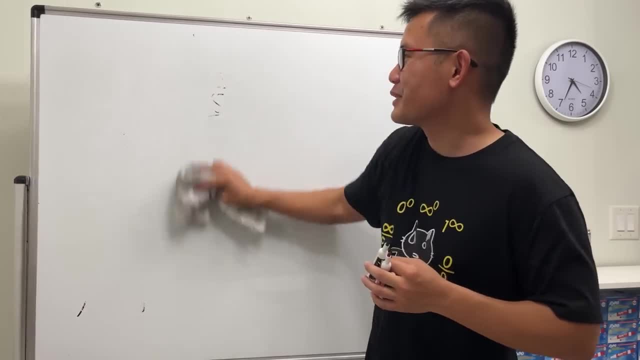 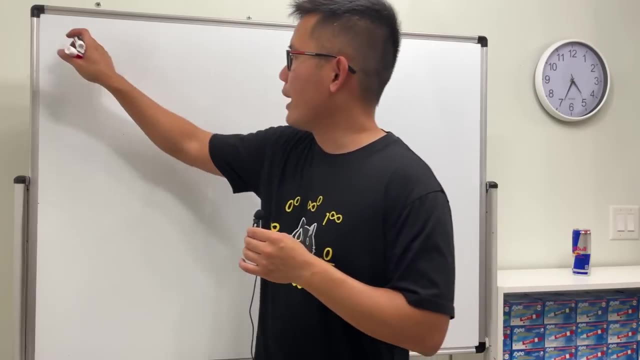 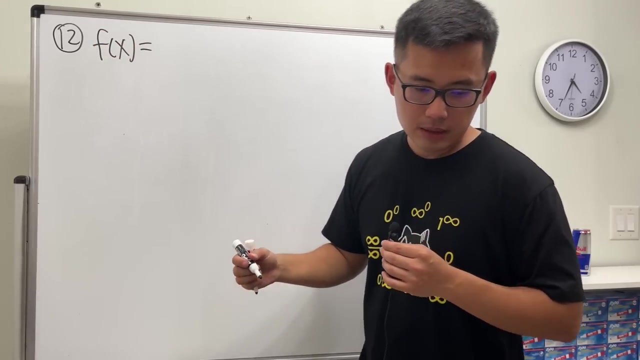 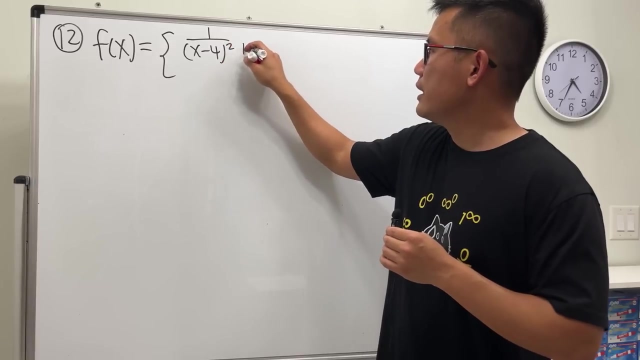 i just do one question and erase. that's why it takes me a long time. okay, number 12.. let me give you guys the function. first, f of x equals again two pieces. first, one, one over x minus four square, and this is when x is not equal to. 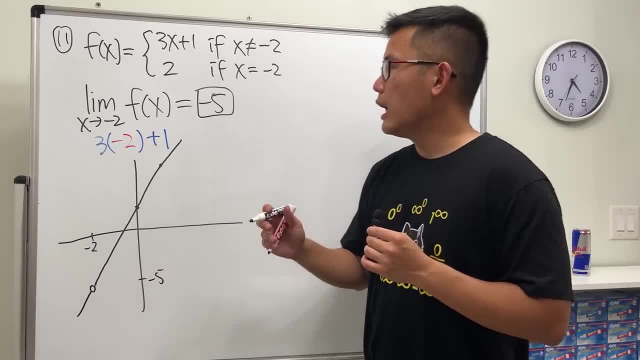 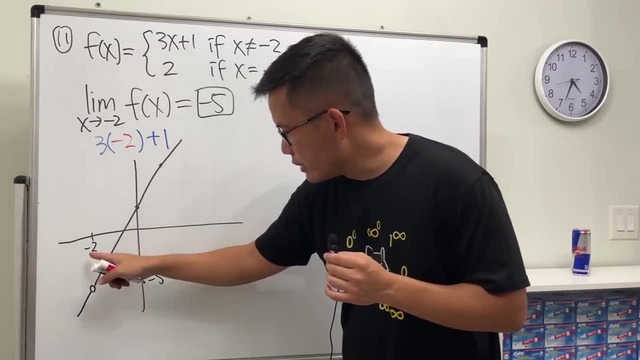 So this right here is negative five. However, We still have to grab the second piece, So we're going to put negative two here. This is the second piece. When x is negative two, the y value is actually at two. So when x is negative two, we actually go up to two. 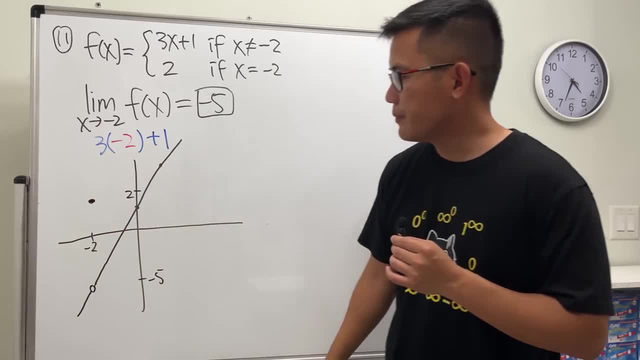 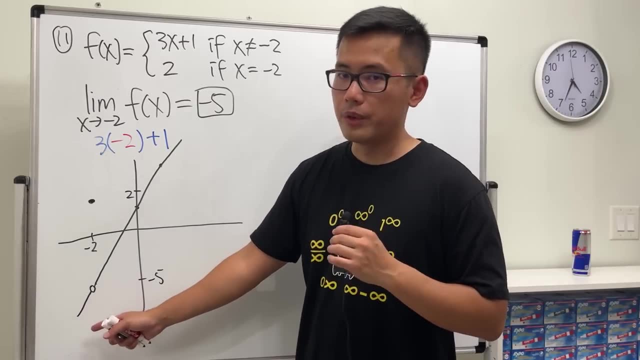 Right here, this is two. Let's say this is two, And then we have a closed circle. So this right here will be the picture for this piecewise function. And now you should be clear that again, just like what we did in the first category, 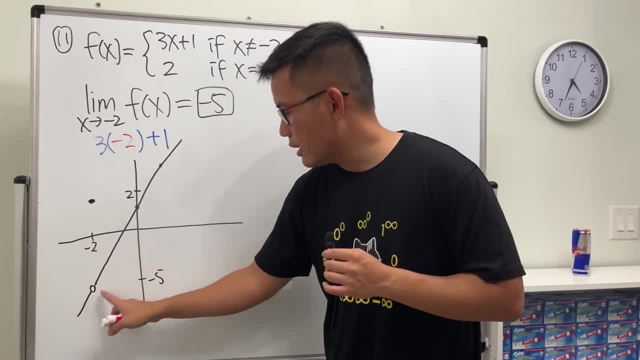 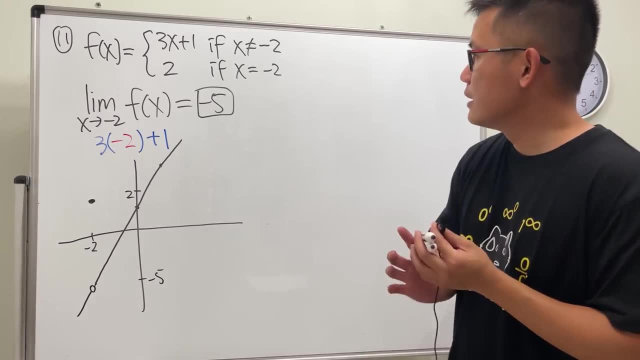 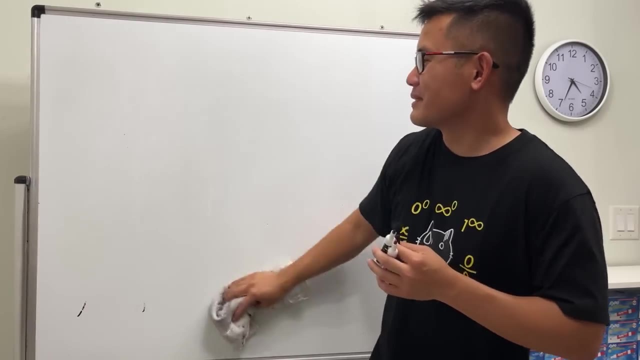 When x is approaching, negative two from the left and from the right. both of them give us negative five. The answer is negative five. Done deal, So that's number 11.. I just do one question and erase. That's why it takes me a long time. 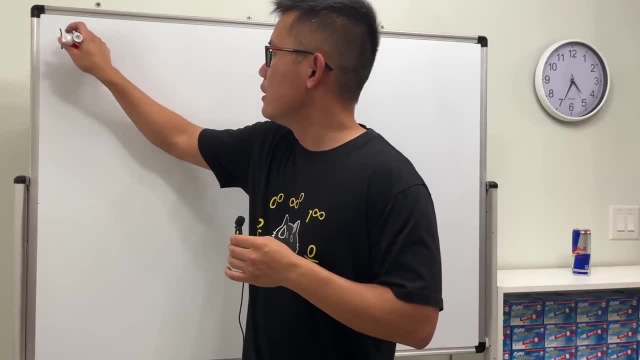 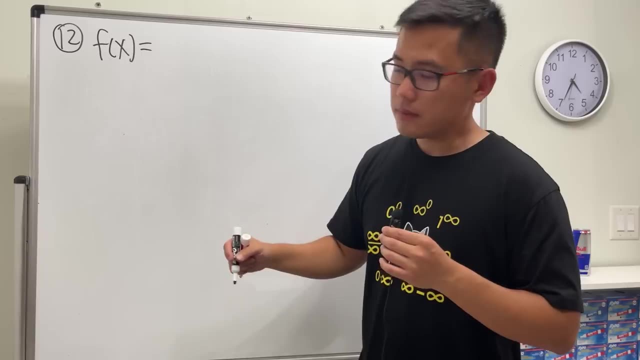 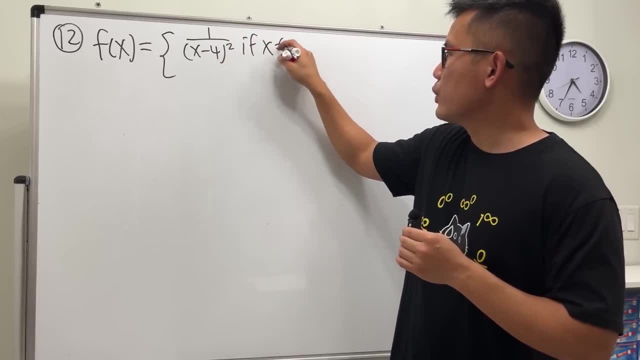 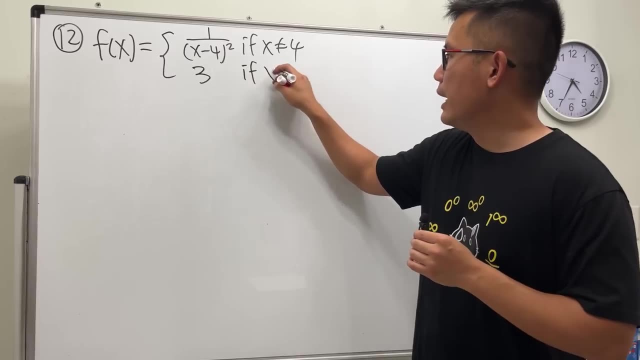 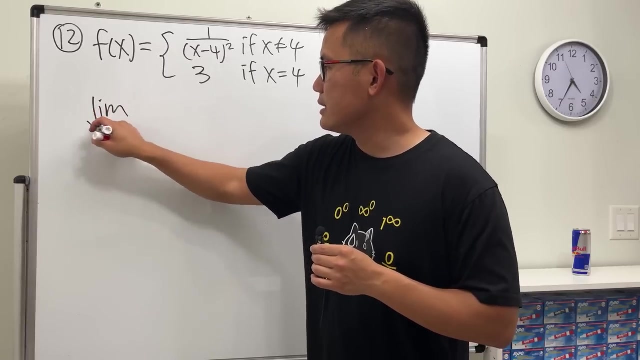 Square, And this is when x is not equal to four And the other one is three. This is when x is equal to four And the question is asking us: what's the limit, as x approaching four, of the function Same deal. 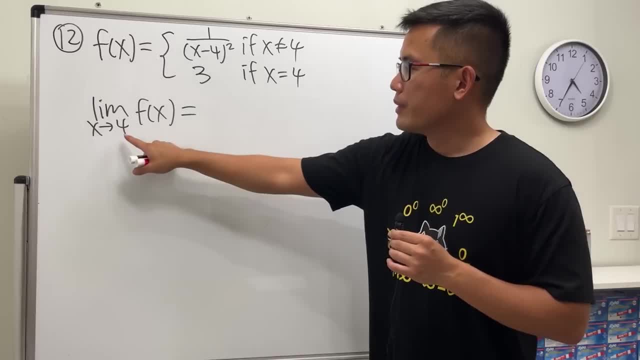 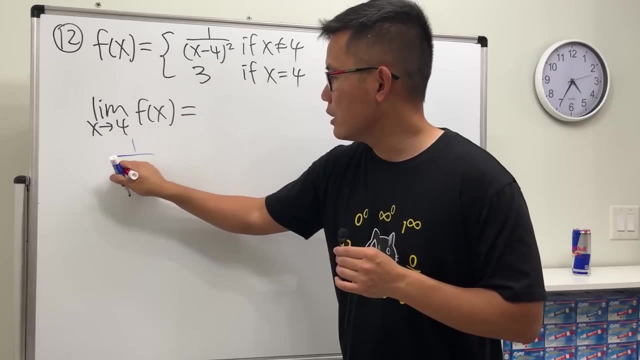 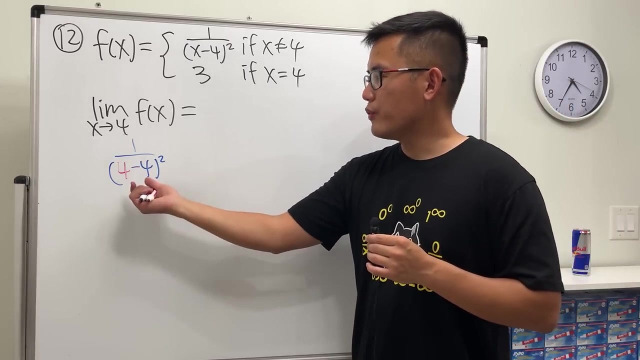 Do not worry about this, because we're talking about limits. So just put four in to here And then let's see, it looks like we are going to get 1 over 4 minus 4, and then square, ah, we get 1 over 0,. unlike earlier, earlier we were able to just find the answer nicely. 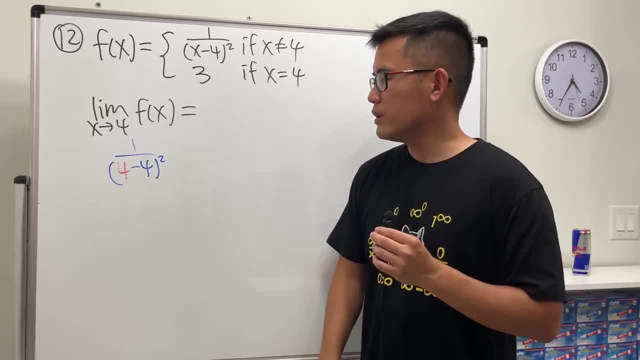 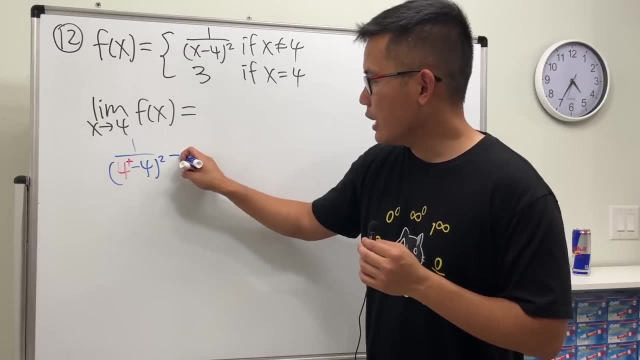 so that's why we didn't have to do the plus or minus. but for this one we should make a better observation. If we have a 4 plus here, okay, that means the x is approaching 4 from the right-hand side. 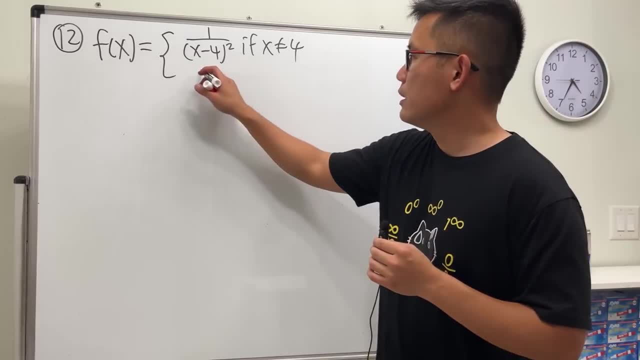 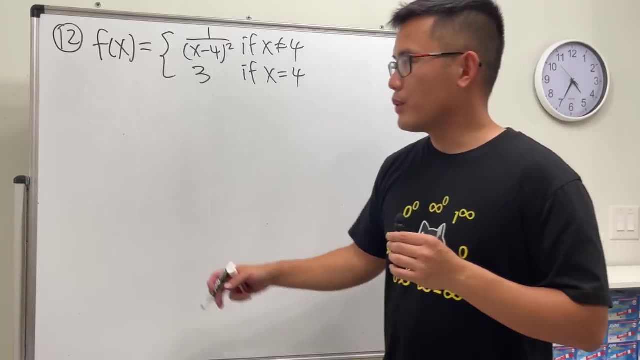 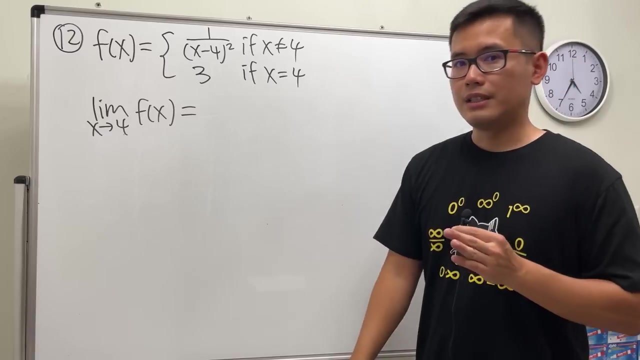 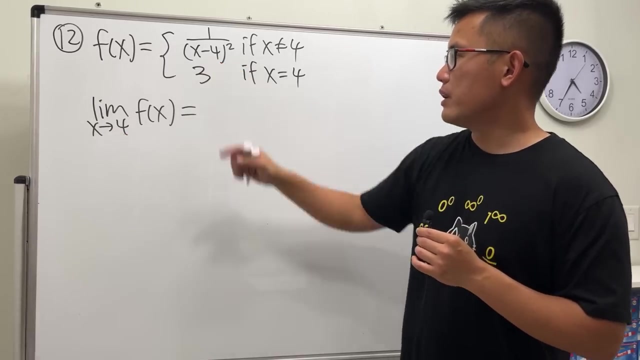 four and the other one is three. this is when x is equal to four and the question is asked: is: what's the limit as x approaching four of the function? same deal. do not worry about this, because we're talking about limits, so just put four into here and then let's see. it looks like we are going. 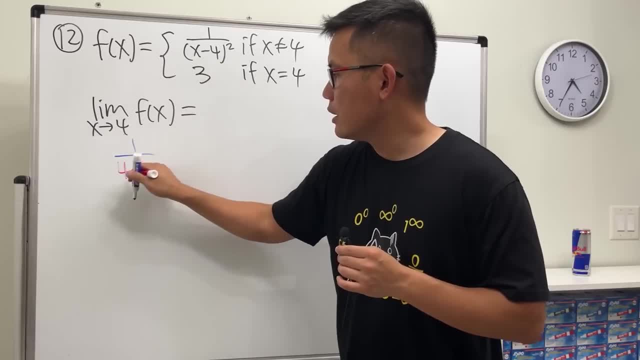 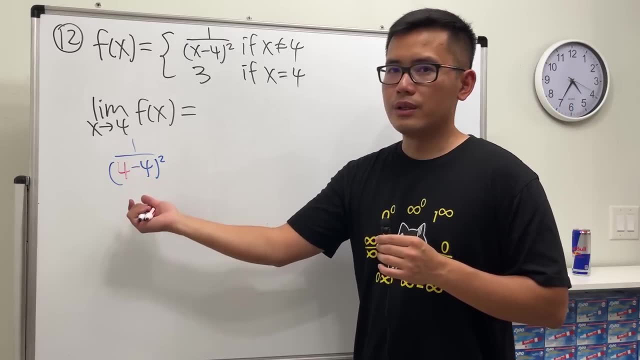 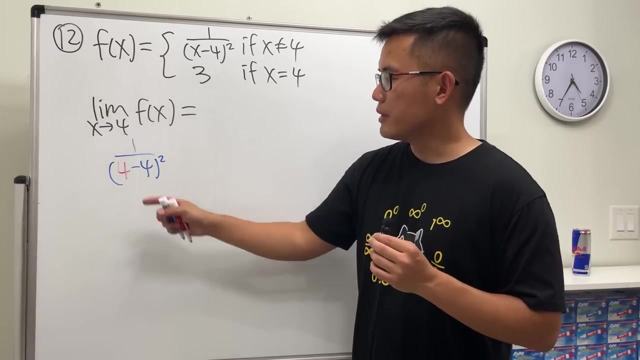 to get one over four minus four, and then square: ah, we get a one over zero, unlike earlier, earlier we were able to just find the answer nicely, so that's why we didn't have to do the plus or minus. but for this one we should make a better. 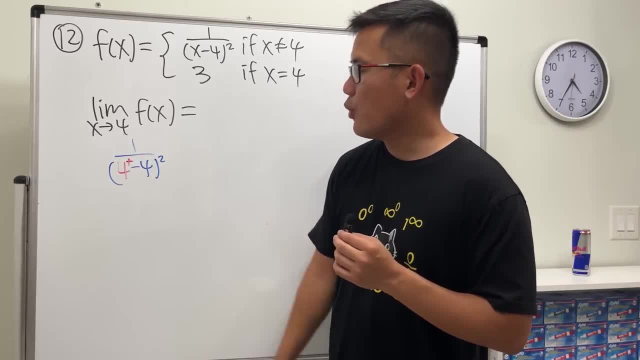 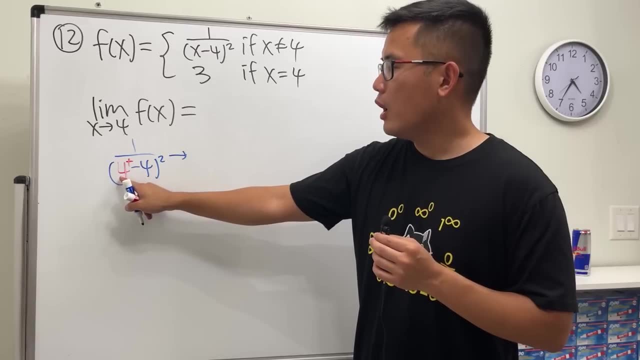 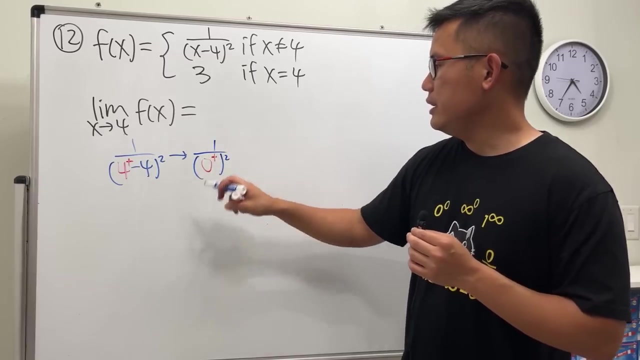 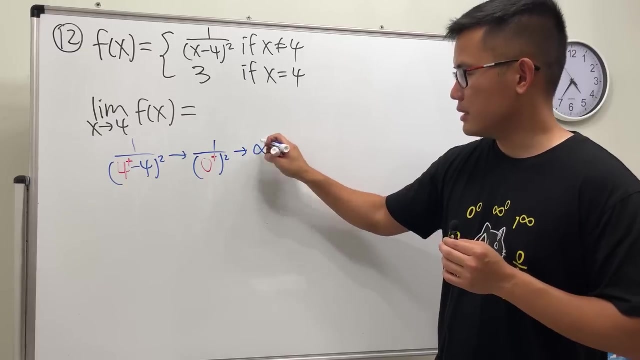 observation: if we have a four plus here, okay, that means the x is approaching four. from the right hand side, four plus minus four, we get zero plus and then square. either way, it's still positive. so, yeah, one over zero and that's a positive. so this right here gives us positive infinity. 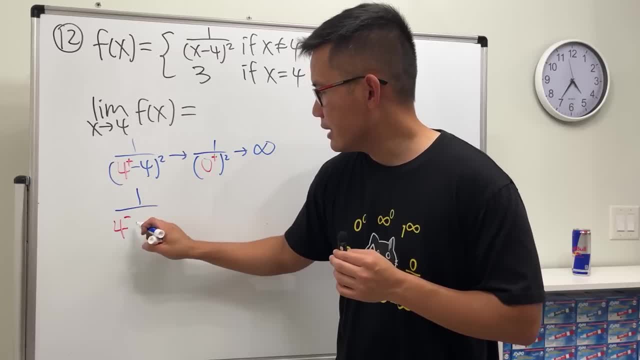 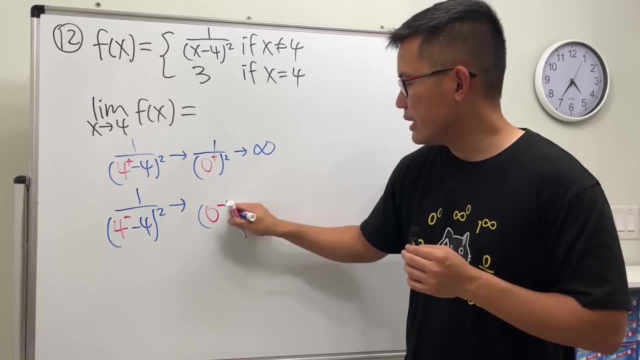 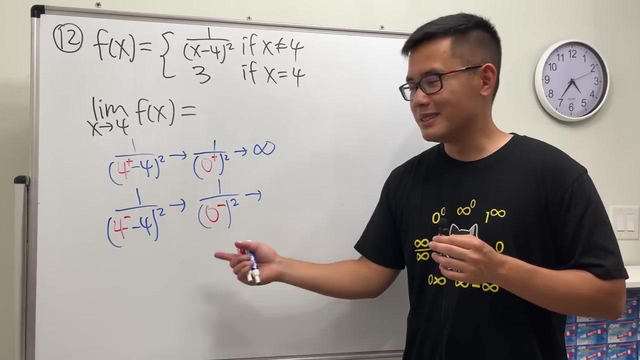 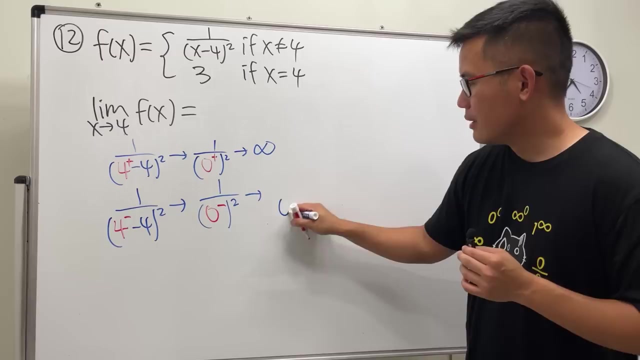 and if we have one over four minus and then minus four inside gives us zero minus, and then we square that. this right here. when we square a negative like zero minus, this is like negative zero, point zero. zero to one, it will give us zero, but it becomes positive, all right. so this right here. 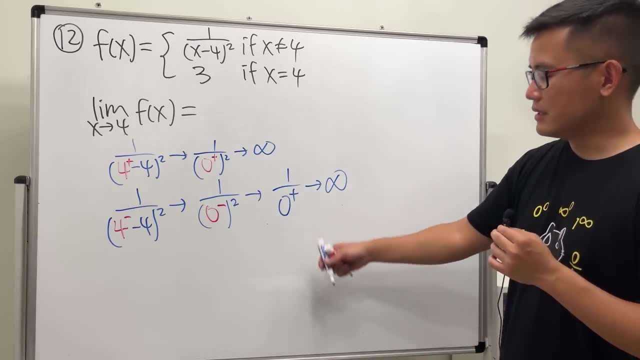 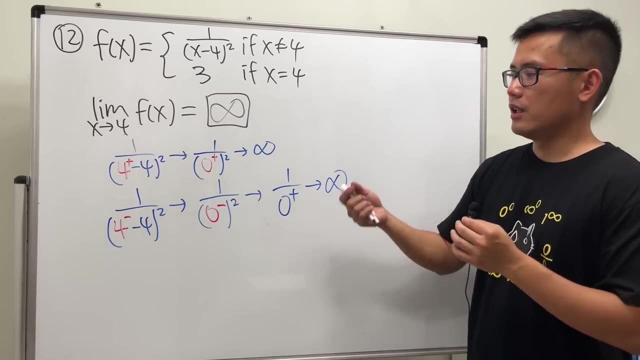 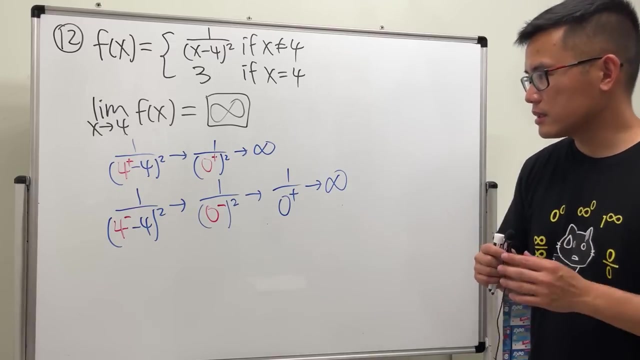 also gives us positive infinity. they are the same. that's why the answer is positive infinity. so this is how you can do it without utilizing the graph: you just kind of write down expressions and then just make arguments or like reason out the answers along the way. so that's pretty good. 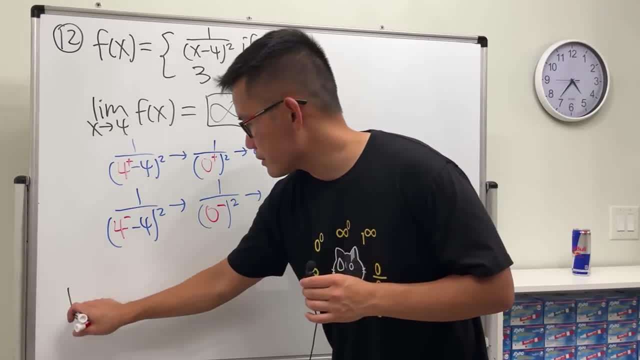 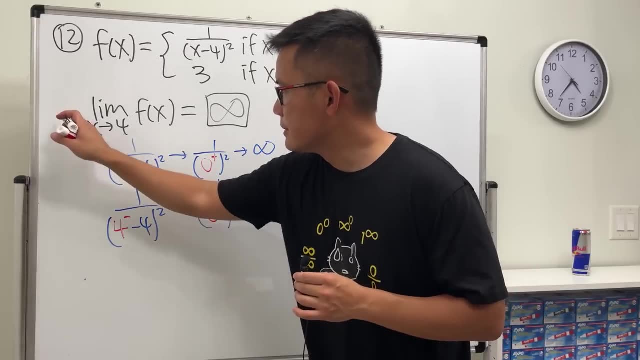 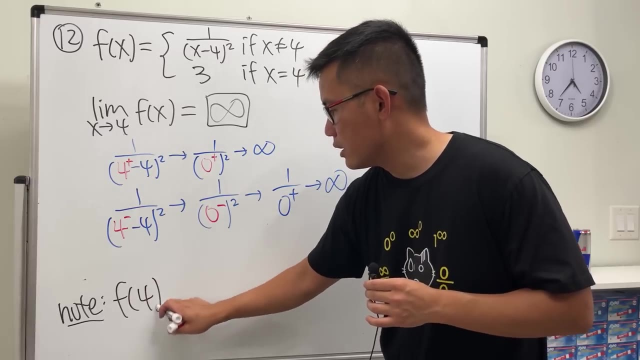 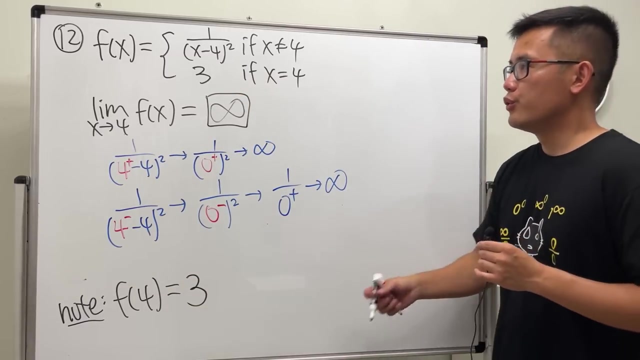 i'll give you guys a picture real quick, though oh, by the way, see, the limit is infinity. uh, if this is part a, i'll give you guys like a popular, like a note on the side f of four. what's the answer for that? f of 4 is 3, right, so just remember all. 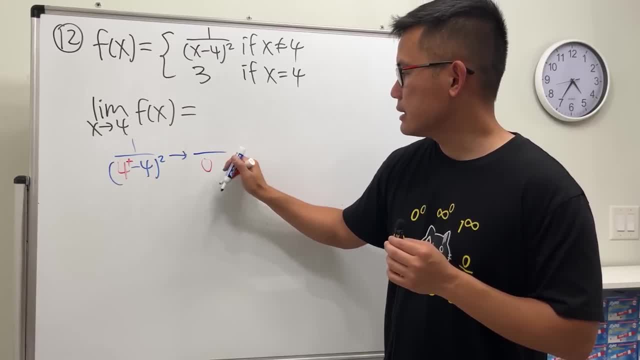 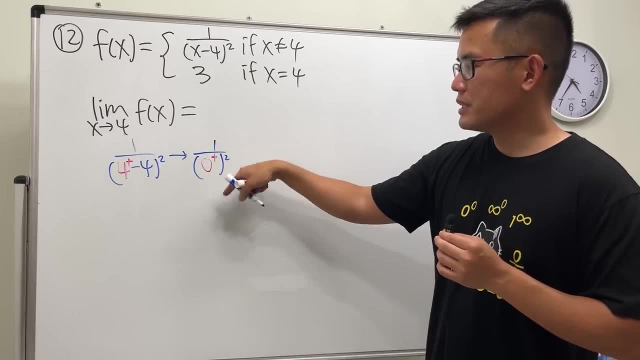 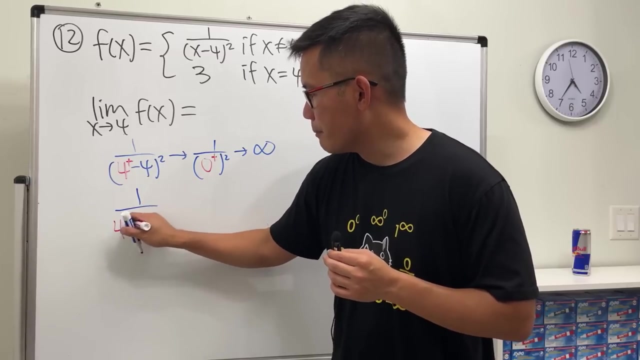 4 plus minus 4, we get 0 plus and then square. either way it's still positive. So, yeah, 1 over 0 and that's a positive. so this right here gives us positive infinity. And if we have 1 over 4 minus, and then minus 4.. 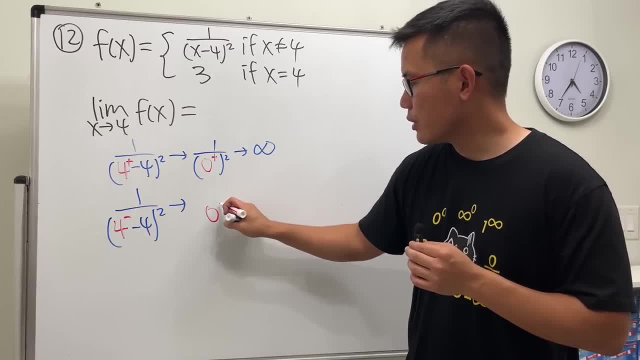 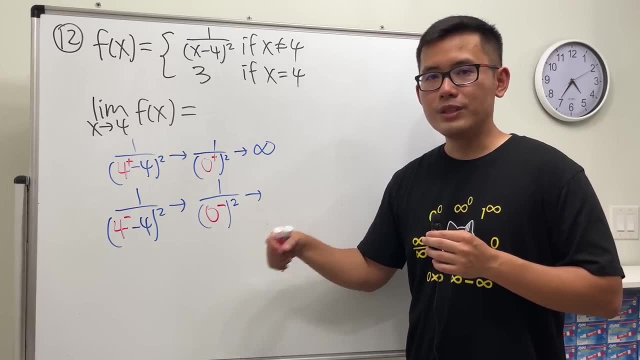 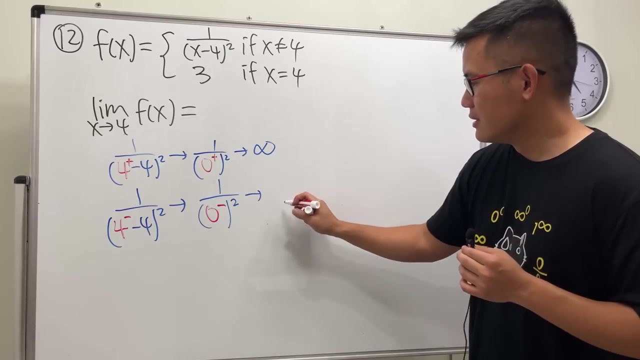 Okay, Inside gives us 0 minus, and then we square that, This right here. when we square a negative like 0 minus, this is like negative 0.0021.. It will give us 0, but it becomes positive alright. 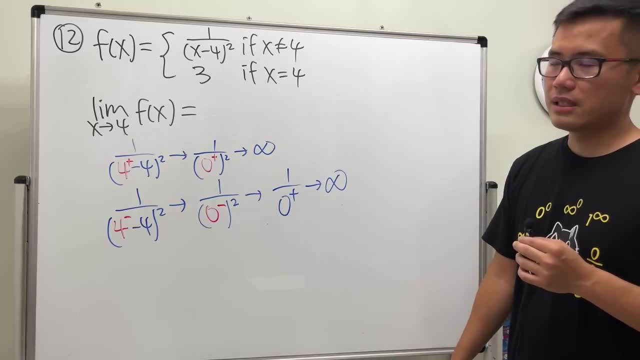 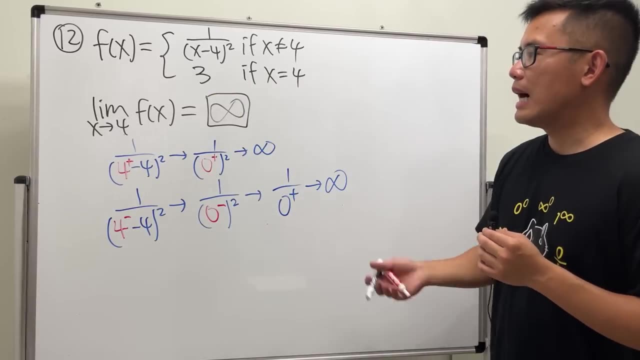 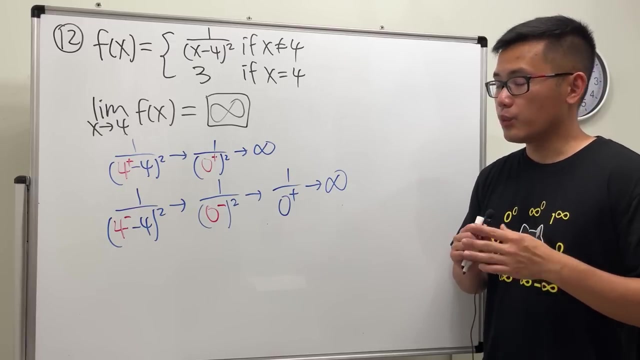 So this right here also gives us positive infinity. They are the same. that's why the answer is positive infinity. So this is how you can do it without utilizing the graph: you just kind of write down the expressions and then just make arguments or like reason out the answers along the way. 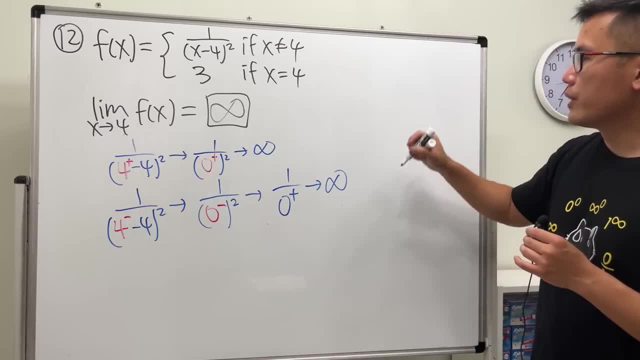 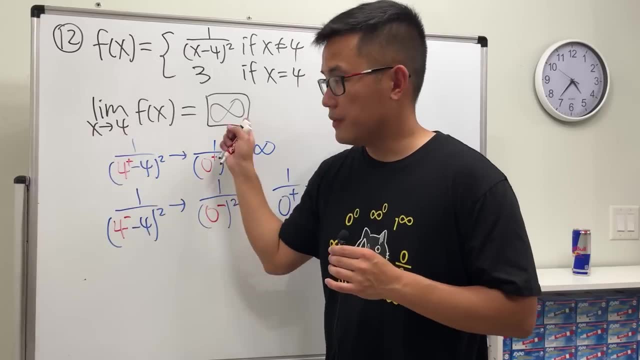 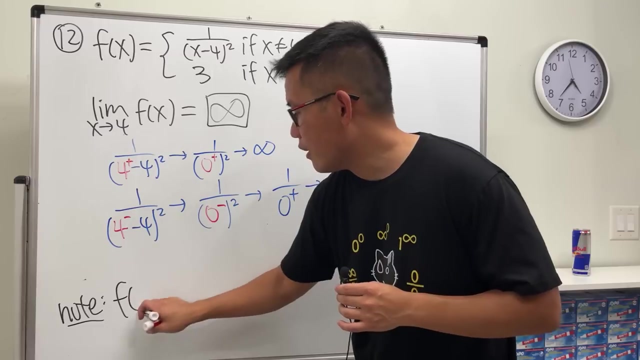 So that's pretty good. I'll give you guys a picture real quick, though. Oh, by the way, see, the limit is infinity. If this is part A, I'll give you guys like a, like a note on the side F of 4.. 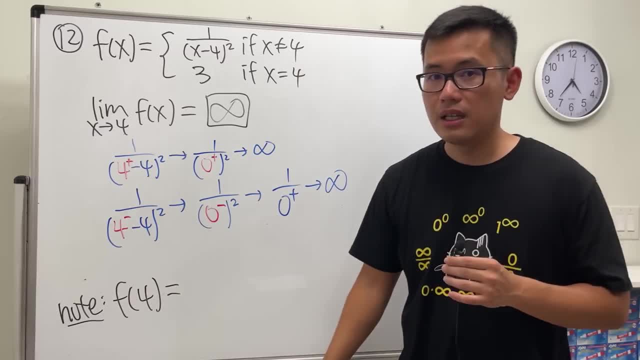 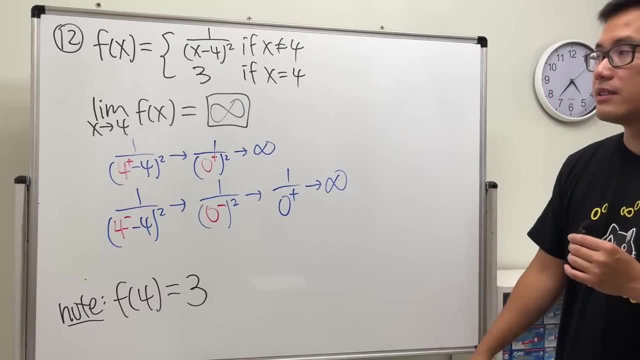 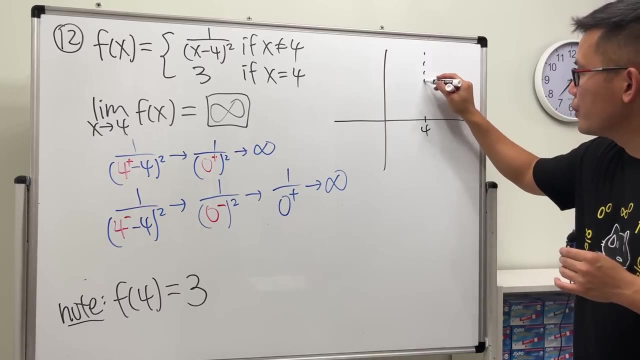 Okay, Okay, F of 4.. What's the answer for that? F of 4 is 3, right? So just remember all the things that we have done so far, And here's the picture. for this, though, X is 4, that's the main value here that we care. vertical isotope, because the bottom. 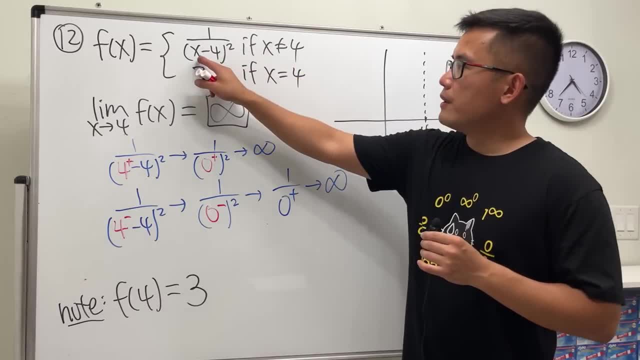 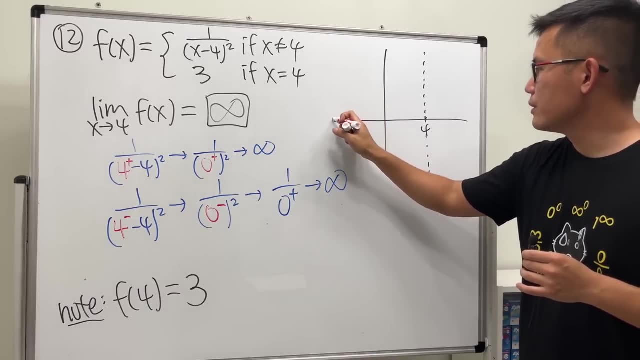 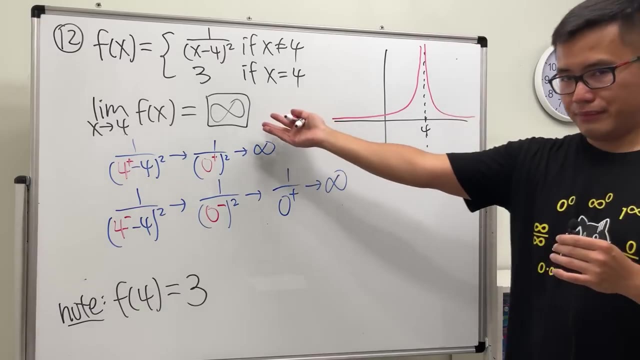 cannot be 0,. huh, 1 over x minus 4 squared it looks like a volcano. So the picture looks like this. I will use red Red to make this one stand out. So like this: like that, that's 1, positive infinity. 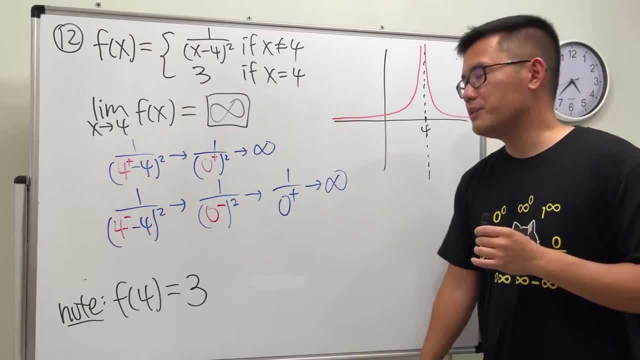 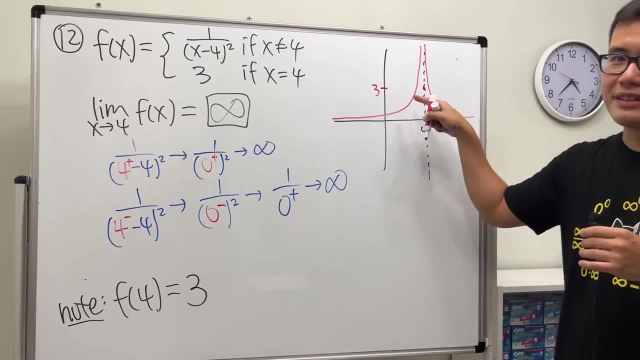 However, not done yet. When x is 4, the y value is 3.. So when x is 4, we should actually go here and then say: let's say this right, here is 3.. So we actually have a dot right there. 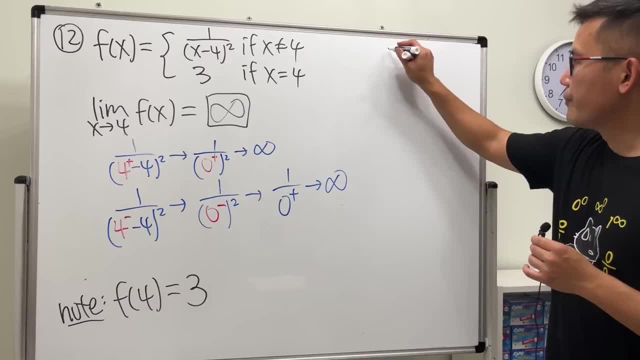 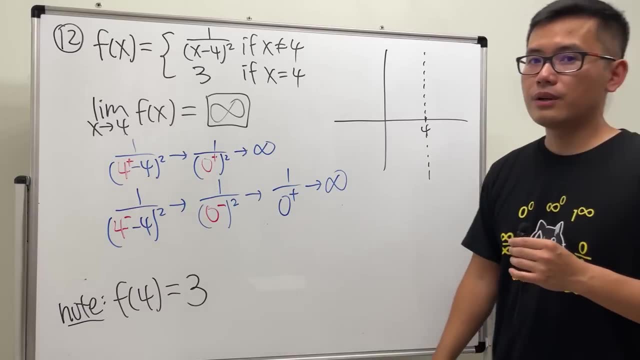 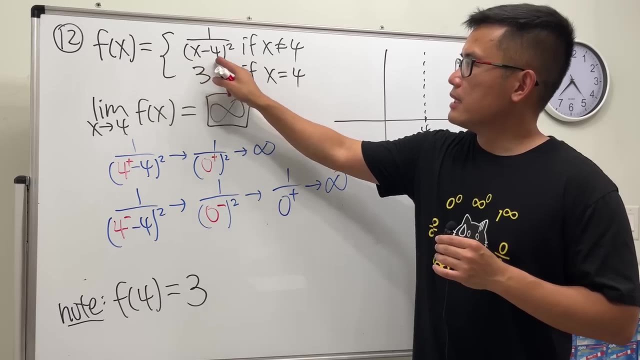 the things that we have done so far. and here's the picture for this, though: x is 4- that's the main value here, that we care- vertical as a top, because the bottom cannot be 0. huh, one over X minus 4 squared, it looks like a volcano. so the picture looks like this. I 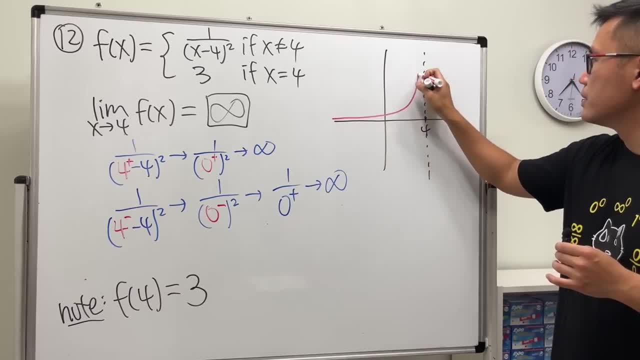 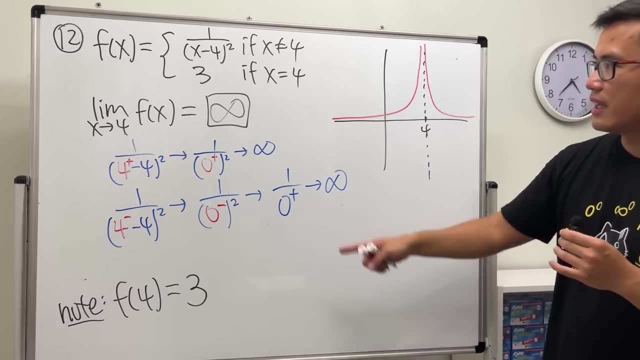 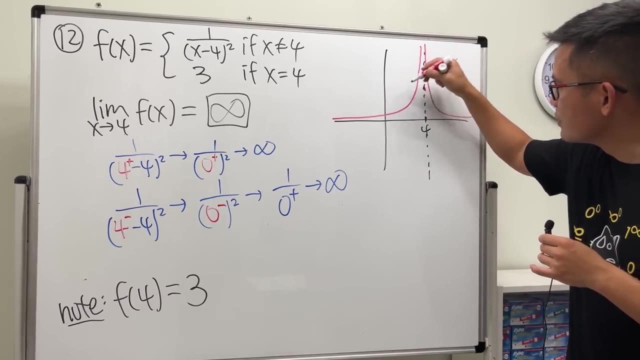 will use red to make this one stand out. so like this, like that. that's why positive infinity. however, not done yet. when X is 4, the y-value is 3. so when X is 4, we should actually go here and say: let's say this right, here is 3, so we. 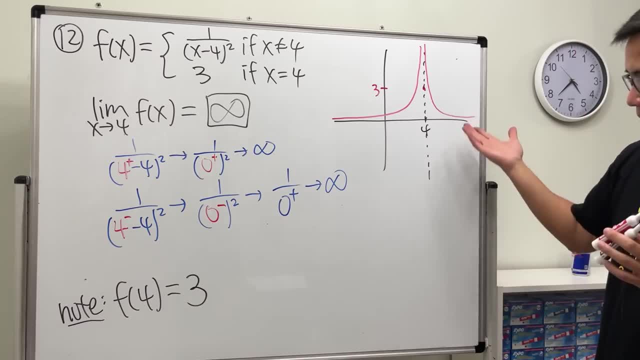 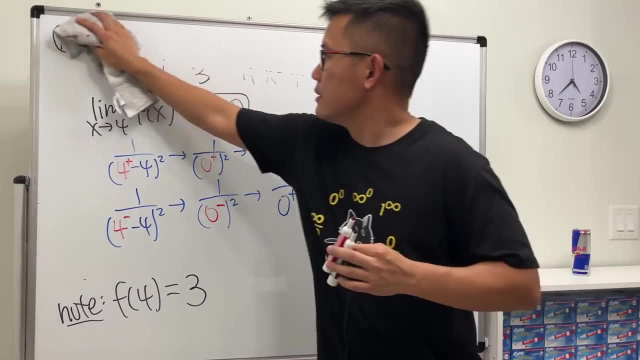 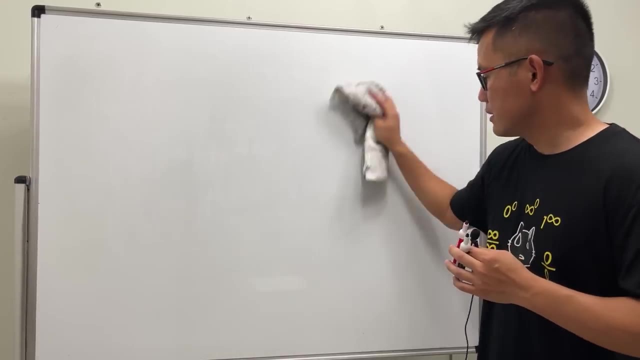 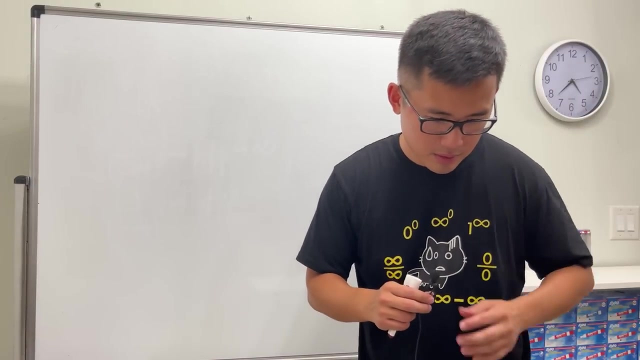 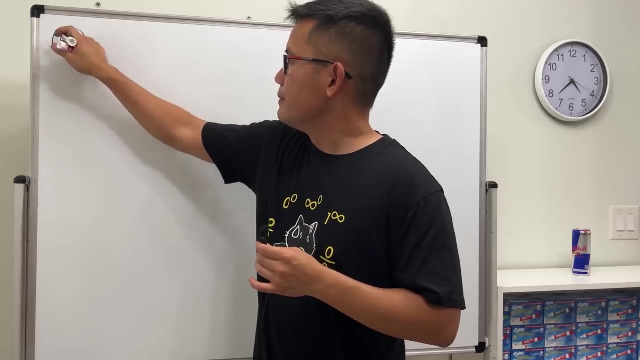 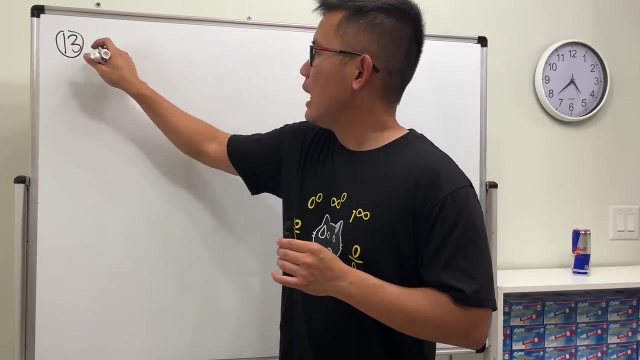 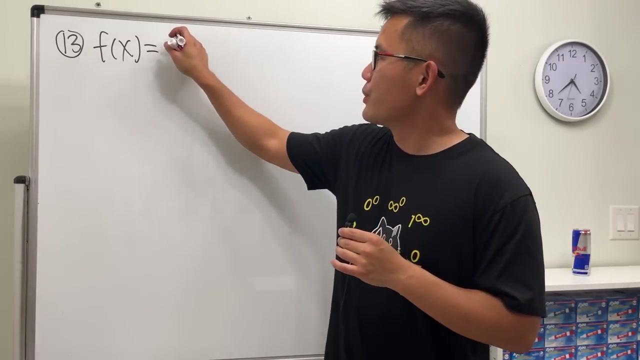 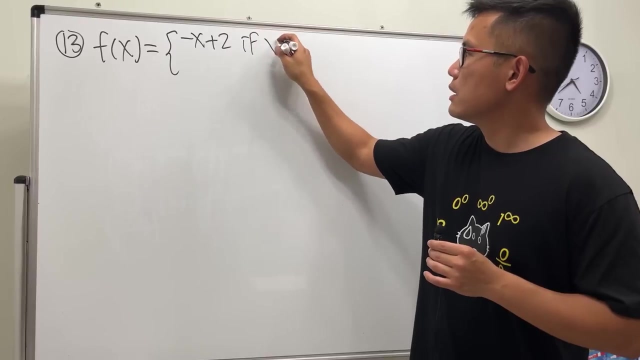 actually have a dot right here. yeah, okay, that's number 12. all right number, just kidding. okay, number 13. our function f of X is equal to a two. two pieces again, don't worry. negative x plus 2, this is when X is less than zero. and then the other one is negative x square plus 2, and this is 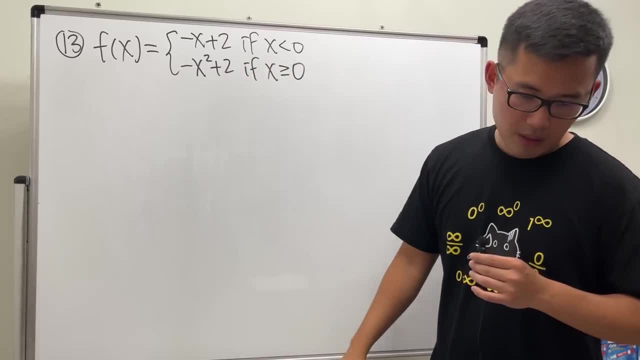 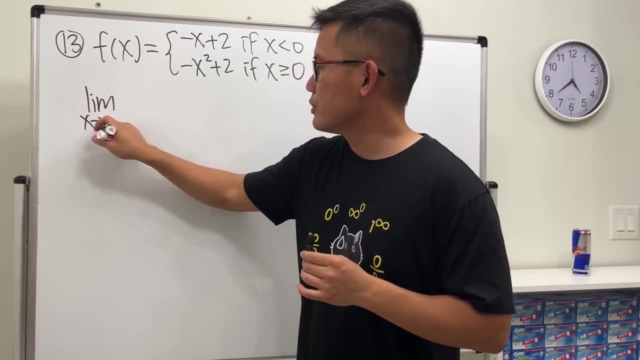 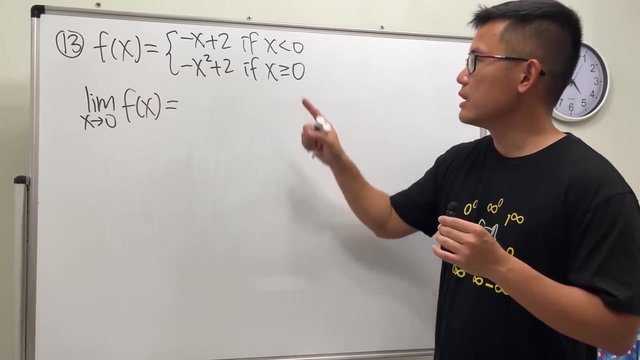 a is greater than or equal to zero, and you can see that zero is the interesting number. so yes, we'll look at the limit as x approaching zero of the function. so for this one we actually have to do left and right because we have the inequality right: x is less than zero and also x is greater. 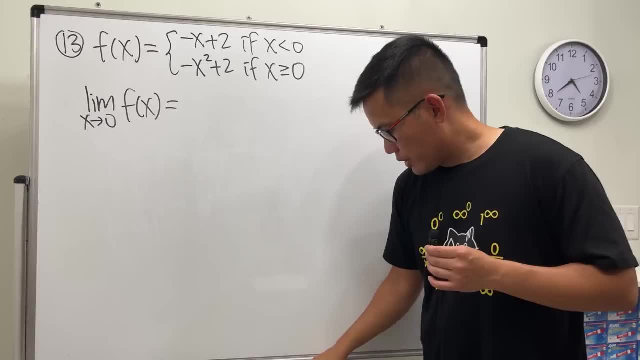 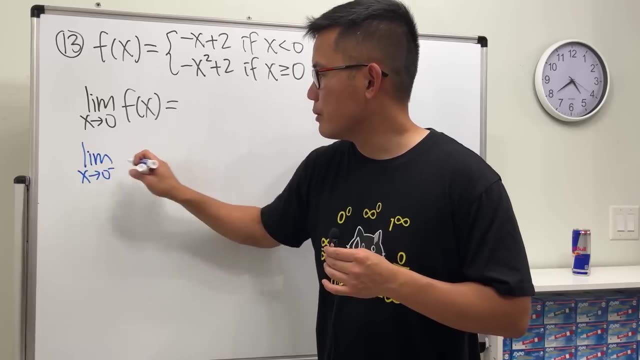 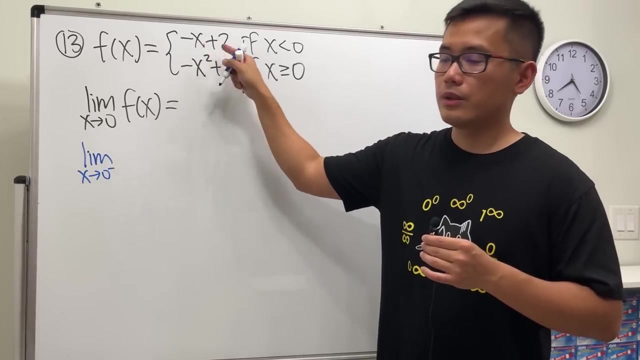 than or equal to zero. so we have a left and right. so here's the deal. let's go ahead and consider. if x is approaching zero minus, let's do that one first. if this is the case, then the function is this piece that we are looking at. so look at negative x plus two, and this is not bad at all. 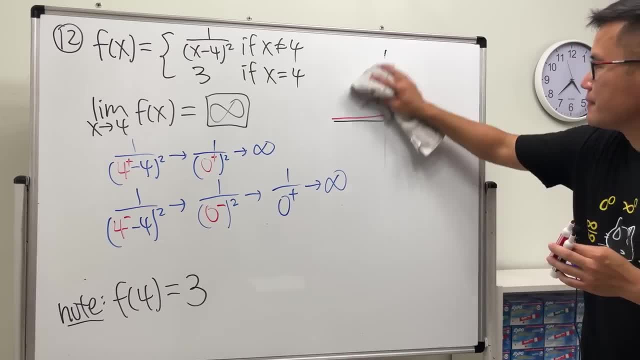 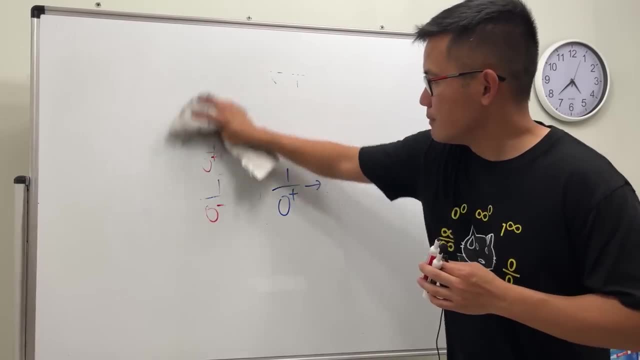 Yeah, Okay, That's number 12.. Okay, That's number 12.. Okay, That's a total of 2.. That's what we want to do, All right, So from here, we're going to add, We're going to add a dot to this function. 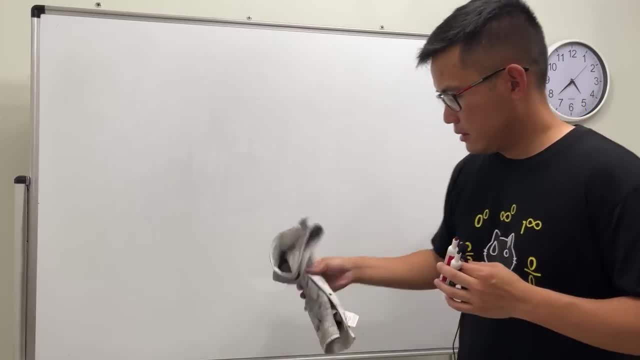 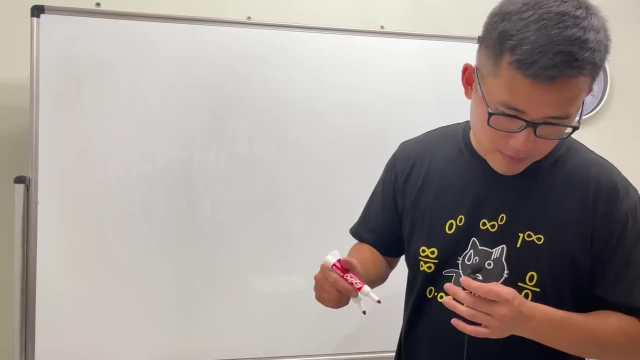 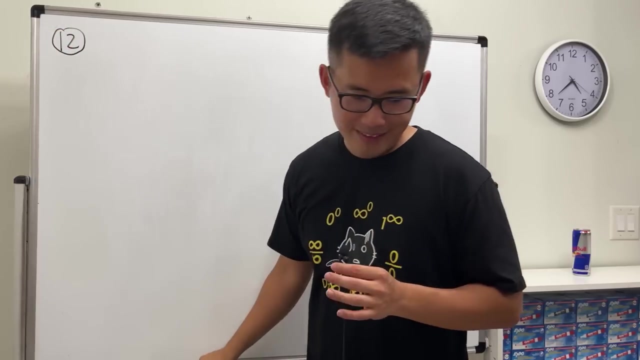 We're going to call this function. We're going to call it function f or log, which is going to be our function. All right Number, Just kidding. Okay, Number 13.. Now that the function f of x is 2, we can say right. 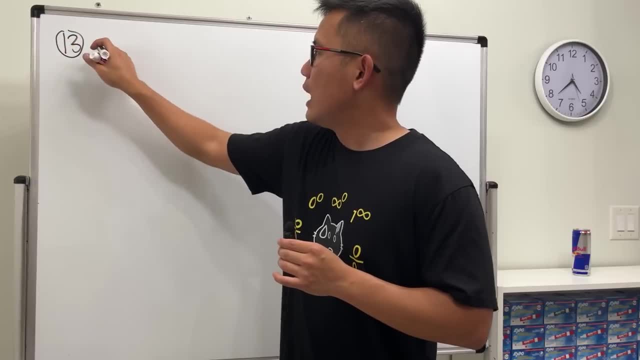 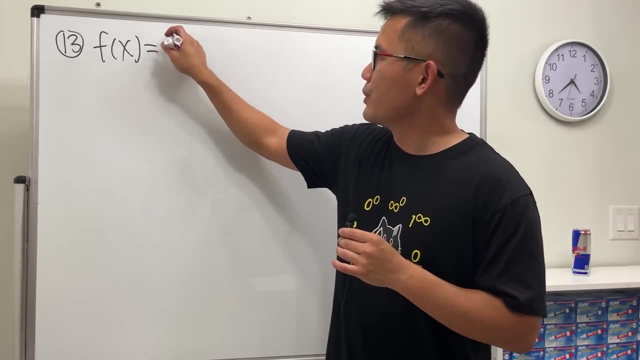 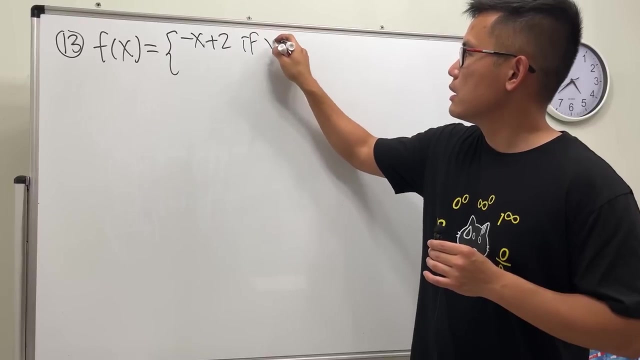 2 over x minus 4. squared, it looks like this thing: our function f of x is equal to: hey, two pieces again, don't worry. negative x plus 2,. this is when x is less than 0, and then the other one is negative x squared plus. 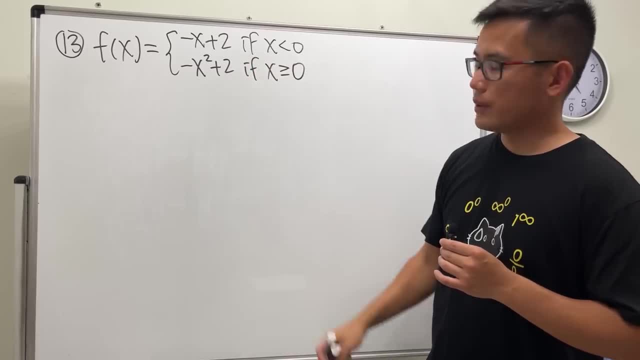 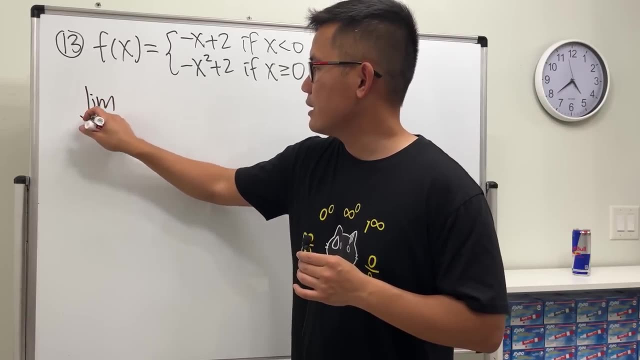 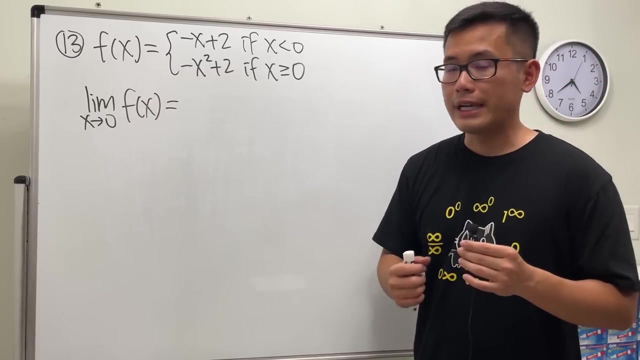 2, and this is if x is greater than or equal to 0, and you can see that 0 is an interesting number. so, yes, we'll look at the limit as x approaching 0 of the function. so for this one we actually have to do left and right because we have the inequality right. x is. 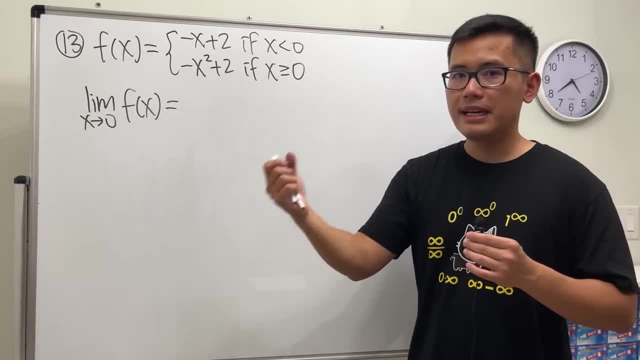 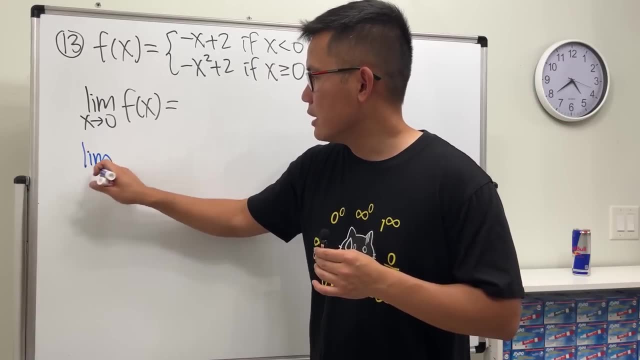 less than 0, and also x is greater than or equal to 0,. so we have a left and right. so here's the deal. let's go ahead and consider. if x is approaching 0 minus, let's do that one first. 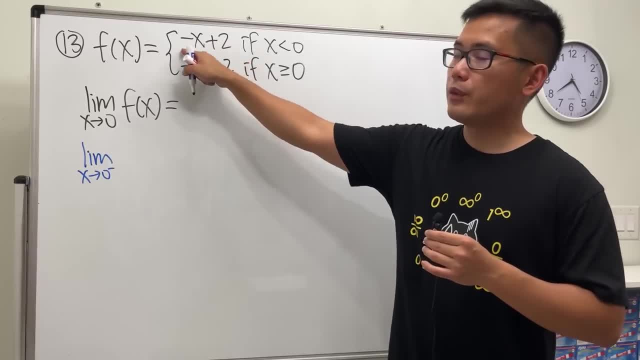 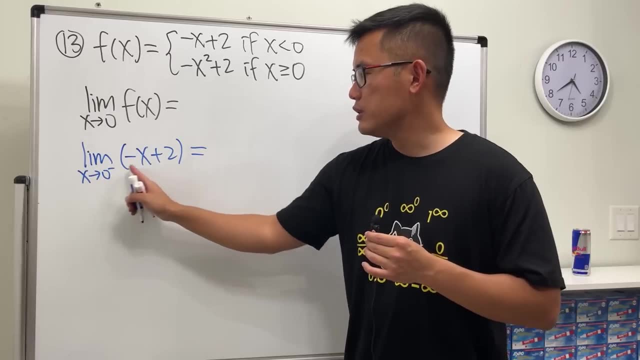 If this is the case, then the function f of x is greater than or equal to 0, and then the function is this piece that we are looking at. so look at negative x plus 2, and this is not bad at all, because if you put 0 in here, this is just going to give us 0, right. 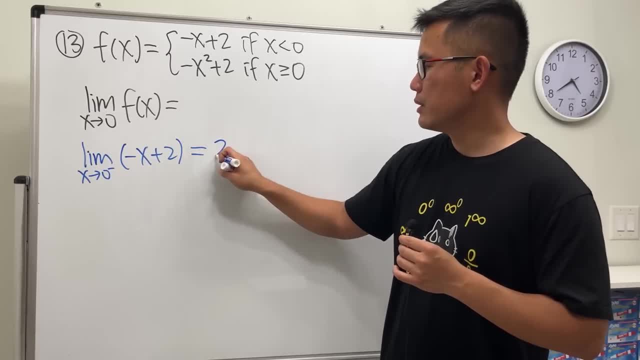 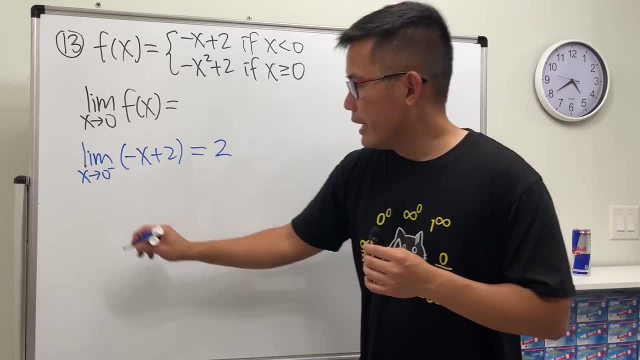 negative 0 is still 0, and then plus 2 is just 2, you don't have to worry about the 0 minus, because plus 2 is just 2, that's the value, that's the limit that we get, and 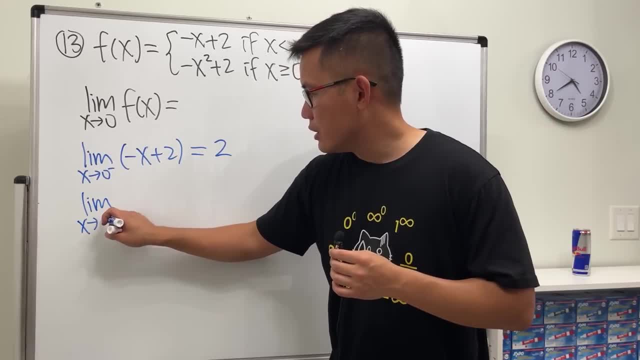 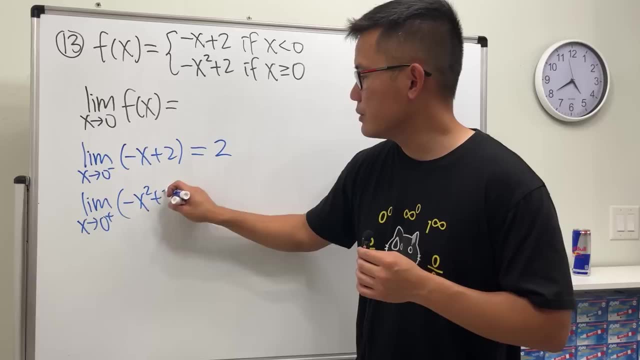 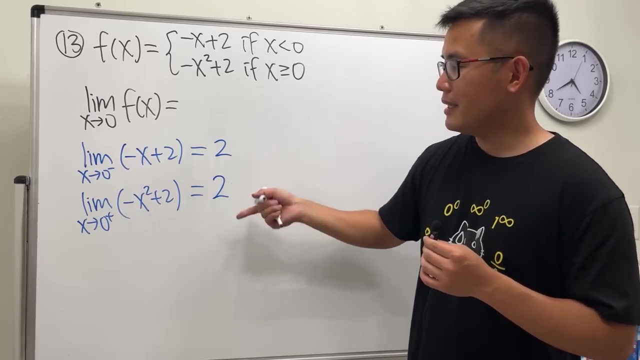 then if we have the limit as x approaching 0, plus, that means x is greater than or equal to 0.. If we look at this piece, which is negative, x squared plus 2, guess what, when we put this right here, that's still 0, plus 2 is still 2, hey, they are the same. that means 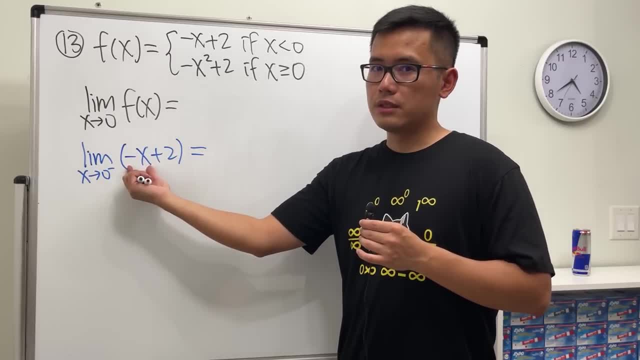 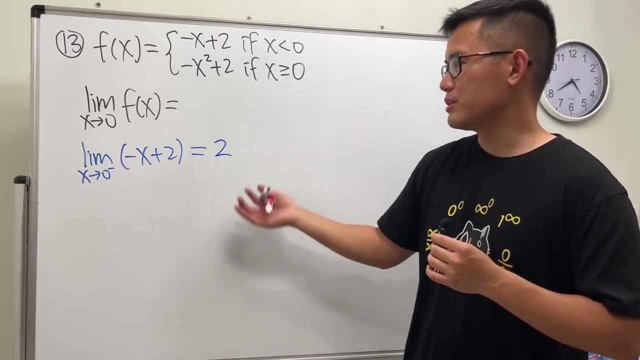 because if you put zero in here, this is just going to give us zero, right, negative zero is still zero. and then plus two, just two. you don't have to worry about the zero minus, because plus two, just two. that's the value, that, that's the limit that we get. 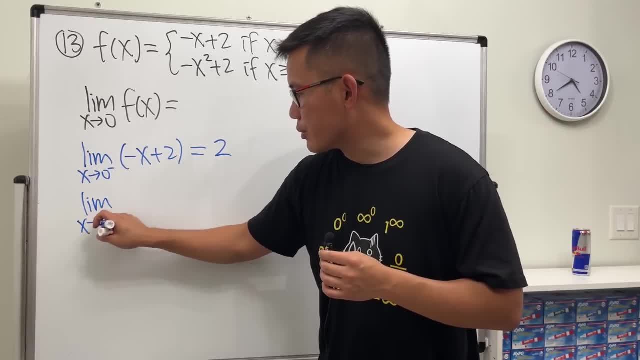 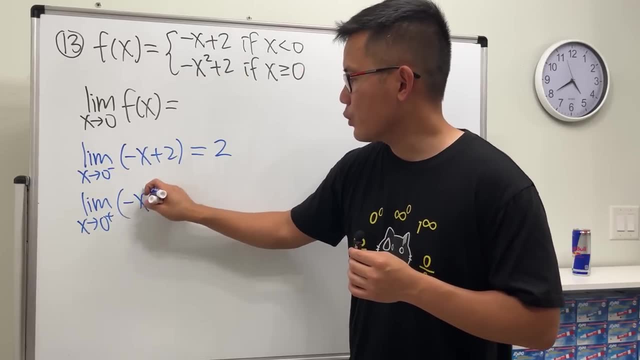 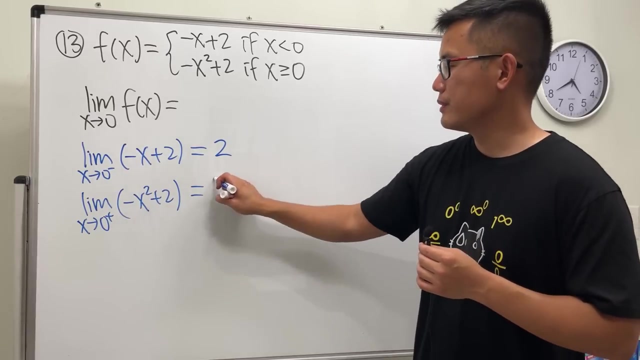 and then if we have the limit as x approaching zero plus, that means x is greater than or equal to zero. we look at this piece which is negative: x squared plus two. guess what, when we put this right here, that's still zero plus two is still two. hey, they are the same. that means when x is. 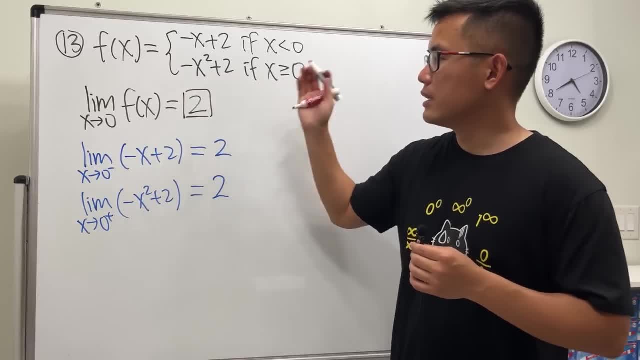 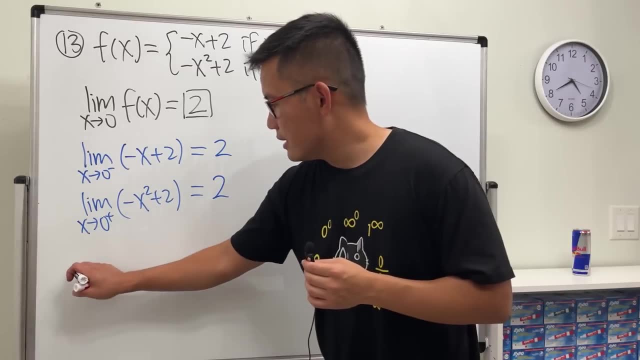 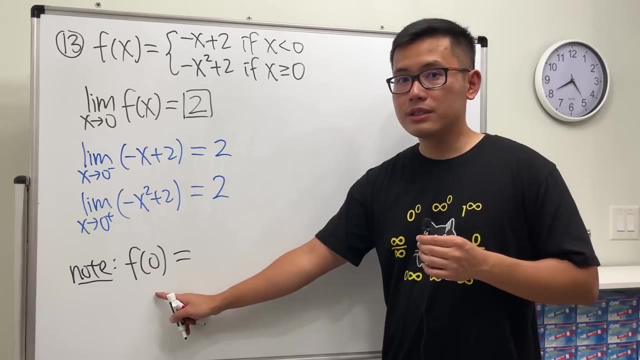 approaching zero of the function, we just get two done. deal, all right. yeah, okay. and then this case i also like to tell you. it happens to be that when we have f of zero, how do we do this? pay attention to the equality: x is equal to zero, right here? 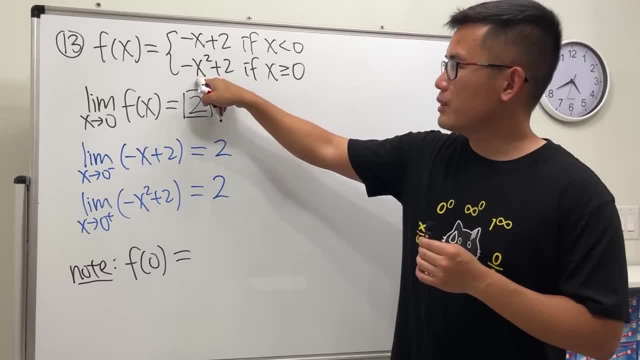 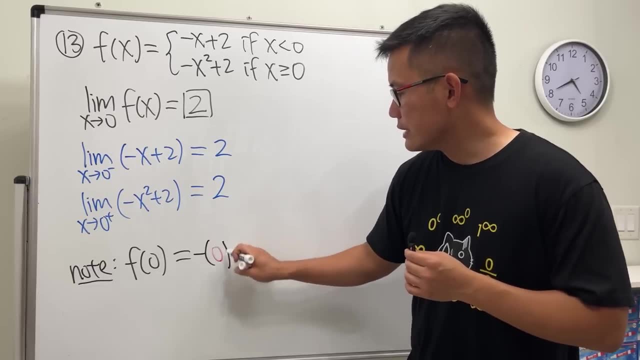 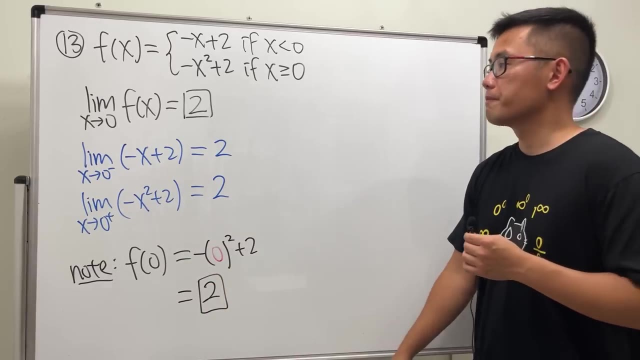 x is greater than or equal to zero, so utilize this one. so for we have this, we technically will have to do negative zero square plus two and work that out. f of zero is two, if that was the question. okay, a picture real quick for this curve. technically it's a line and a curve. 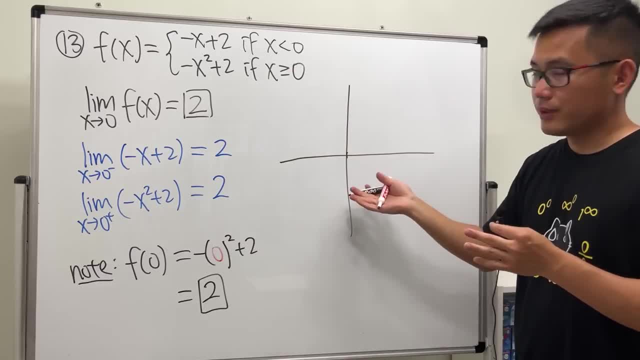 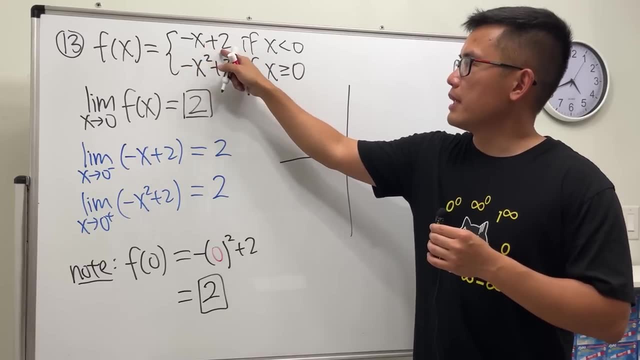 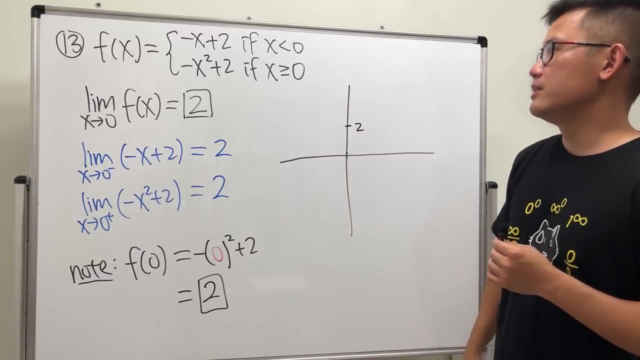 zero is the like, an endpoint, so pay attention to that. when x is less than zero, we do this, which is just the equation of a line: negative x plus two. two is the y intercept. so we have it up here and let's say this: right, here is two. and then negative x is just. 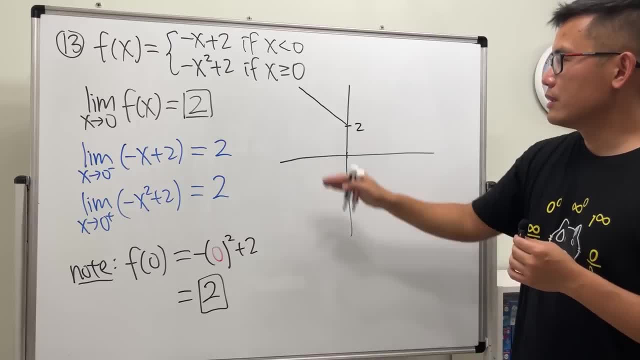 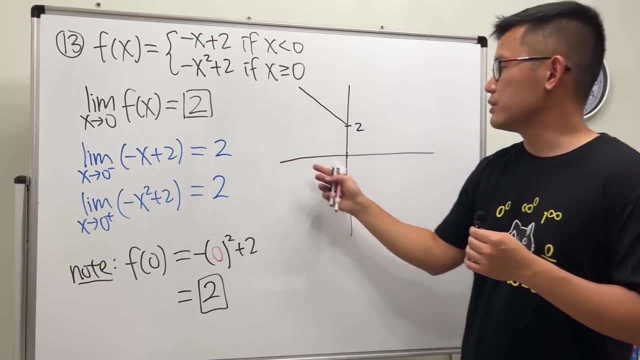 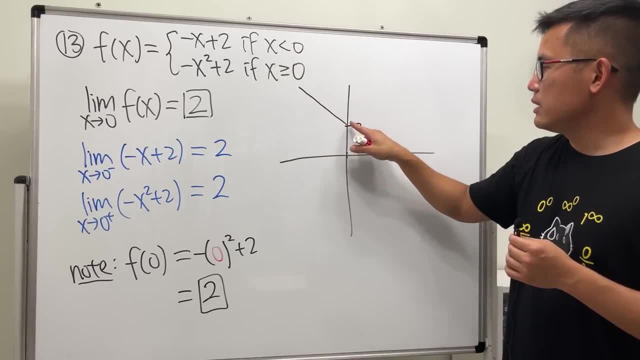 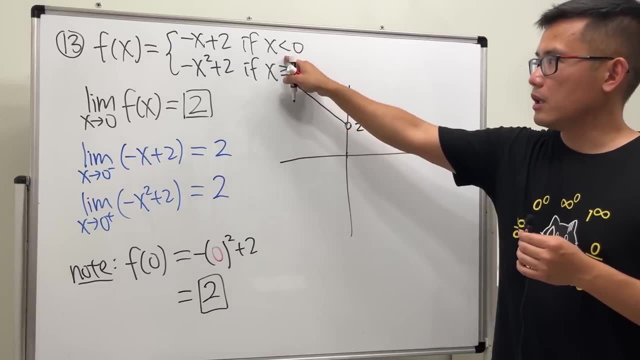 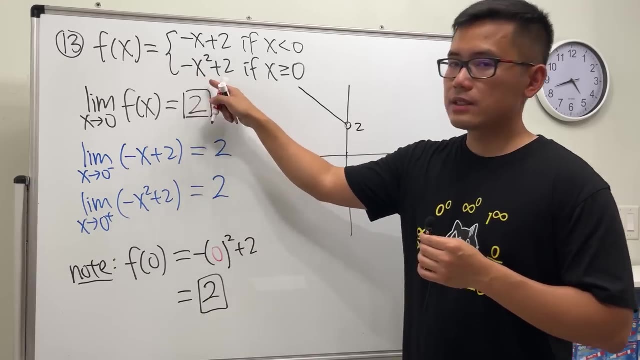 point. however, this is x less than zero, so technically i should have put an open circle here. i'm just doing this in order. so open circle because of this inequality. and then for the second part, we have this parabola: negative x squared is like this: right. 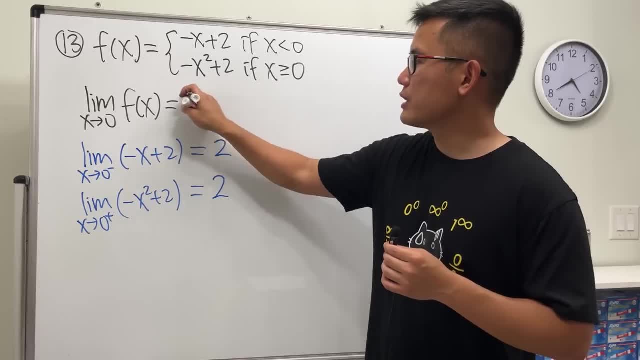 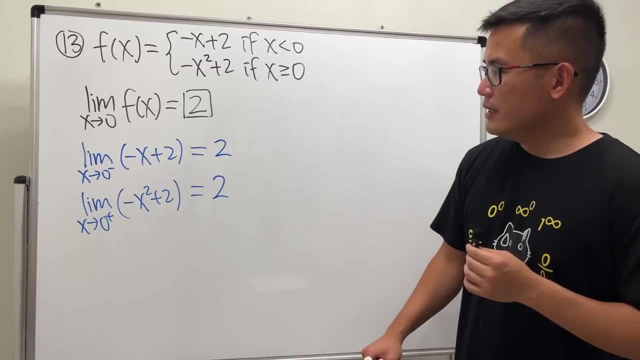 when x is approaching 0 of the function, we just get 2, done deal, alright, yeah, okay. and then this case I would also like to tell you. it happens to be that when we have f of 0. 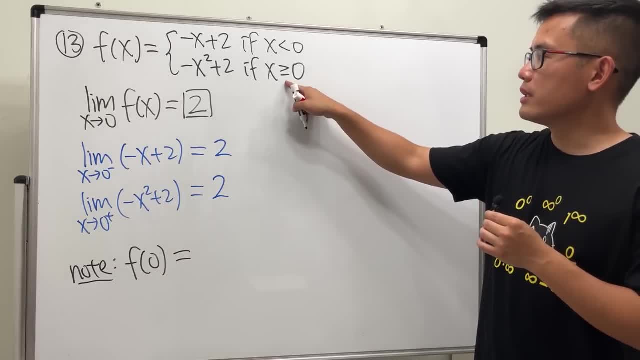 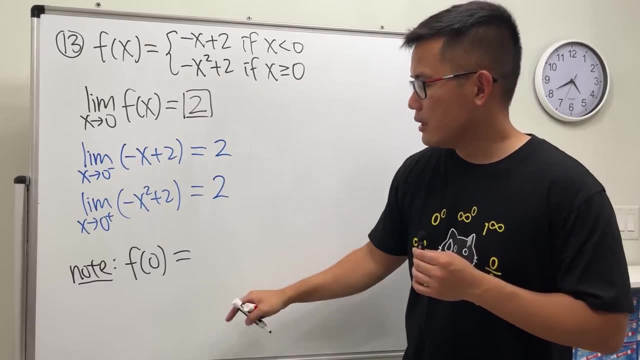 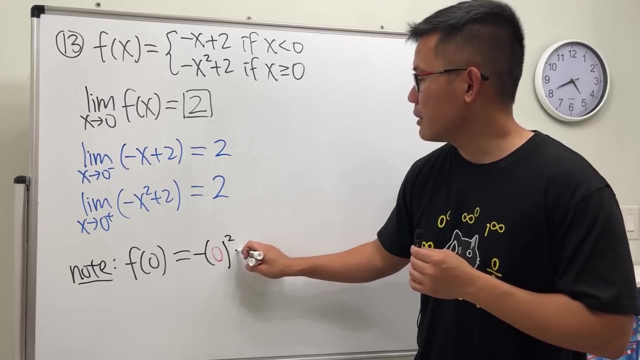 How do we do this? Pay attention to the equality: x is equal to 0, right here, hey, x is greater than or equal to 0, so utilize this one. so for we have this, we technically will have to do negative 0 squared plus 2, and then work that out. f of 0 is 2, if that was the question. 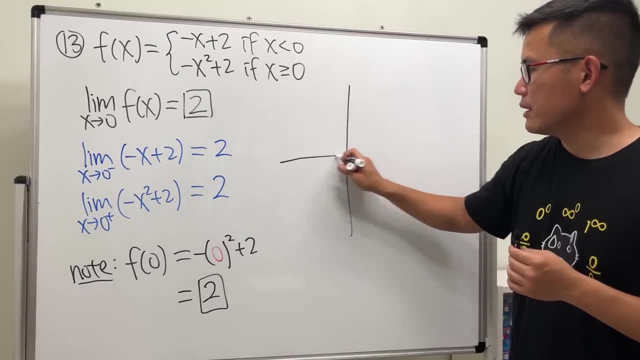 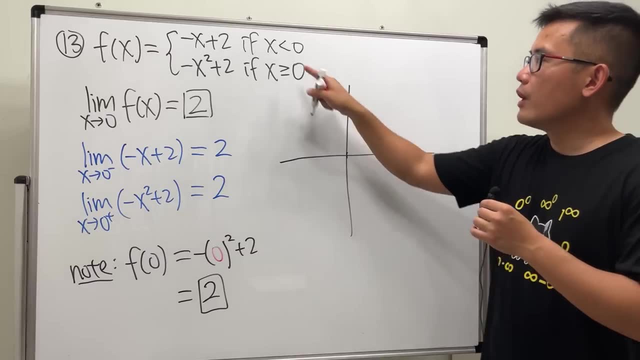 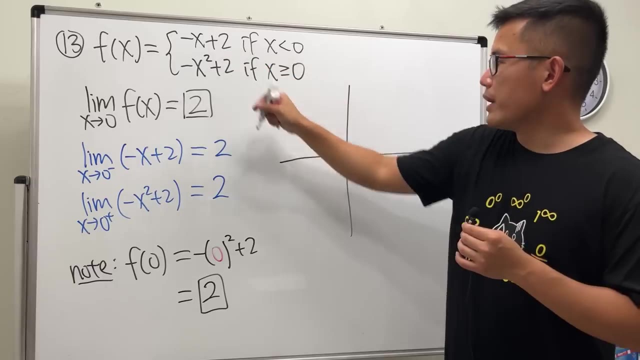 Okay, a picture real quick for this curve. technically it's a line, It's a curve. 0 is the like, an endpoint, so pay attention to that. when x is less than 0, we do this, which is just the equation of a line: negative x plus 2, 2 is the 1 intercept. 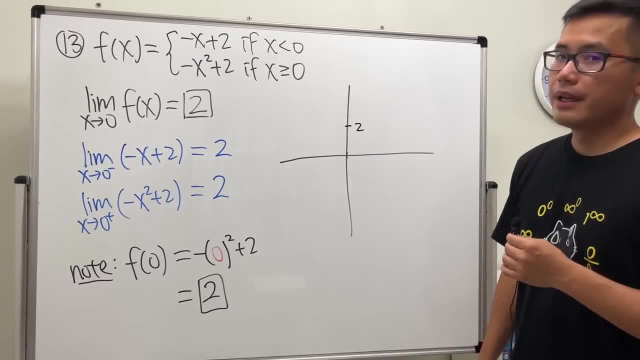 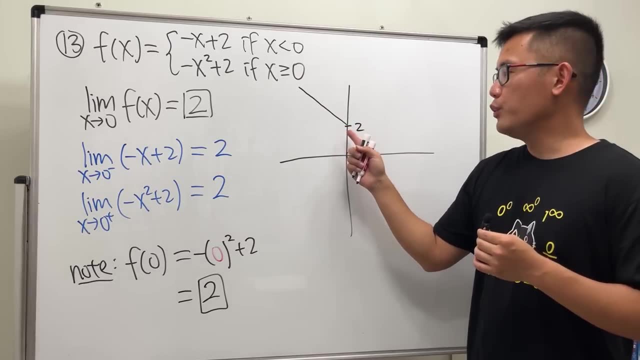 so we have it up here and let's say this: right here is 2, and then negative x is just like this: right the slope, negative 1, or, if you would like, you can just plug in negative 1 in here: negative negative 1 is 1,, 1 plus 2 is 3.. 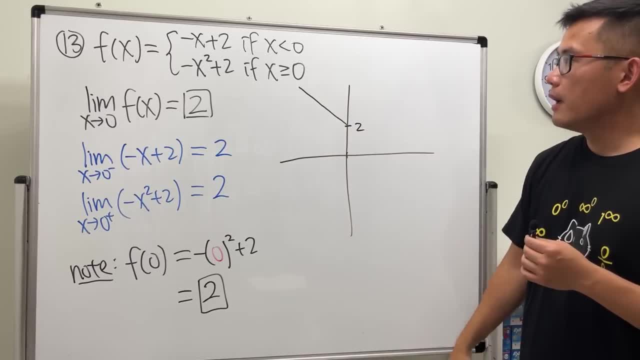 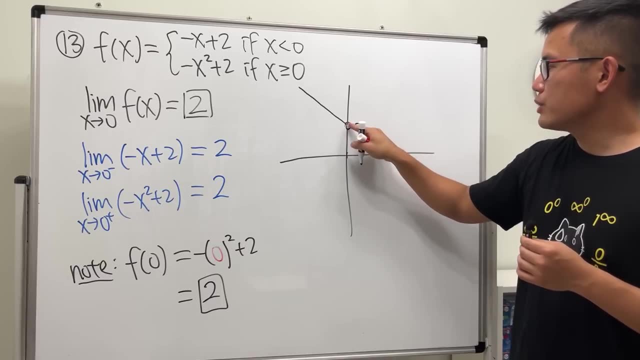 So negative: 1.. 1,, 3, and you have another point. However, this is x less than 0, so technically I should have put an open circle here. I'm just doing this in order. so open circle because of this inequality and then for the 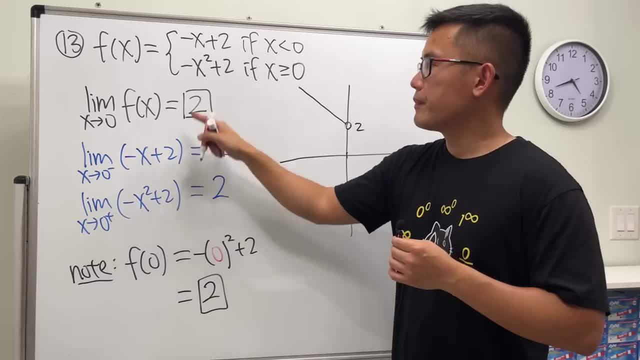 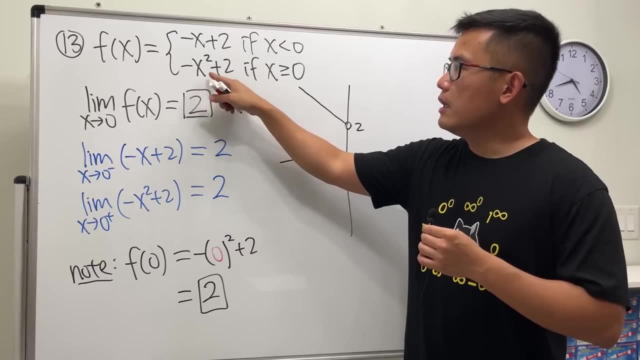 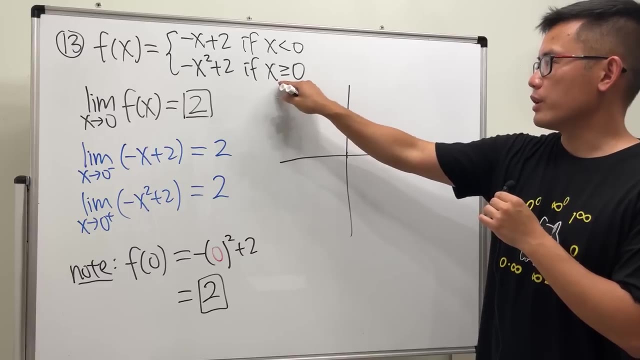 second part. we have this parabola: negative x squared is like this: right upside down parabola. however, it's been shifted up two units. it happens to be here and just the right-hand side, Because that's only when we have x is greater than or equal to 0.. 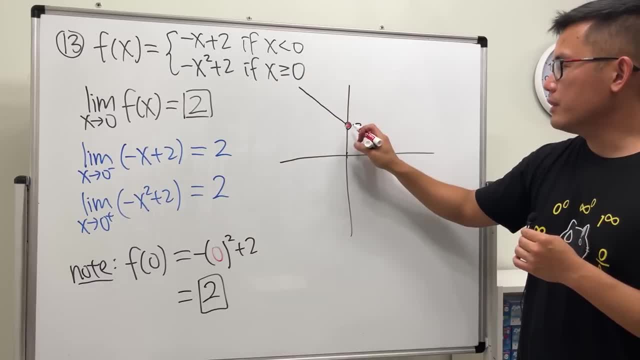 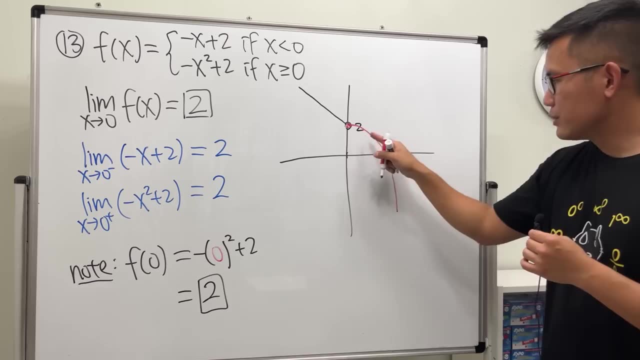 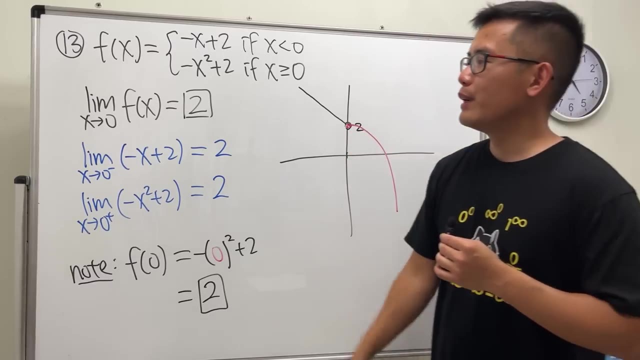 So we start it right here because, thanks to equality here and then we have a parabola. So this right here is the line, this right here is the parabola, and you can see that the function is continuous when x is equal to 0, that's why the limit and the value of 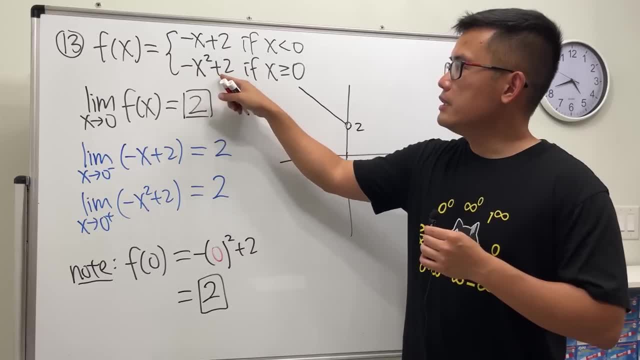 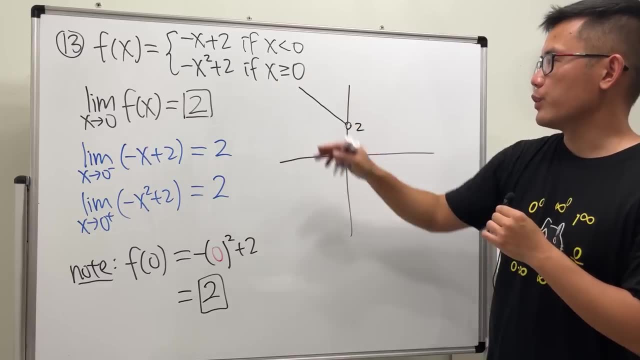 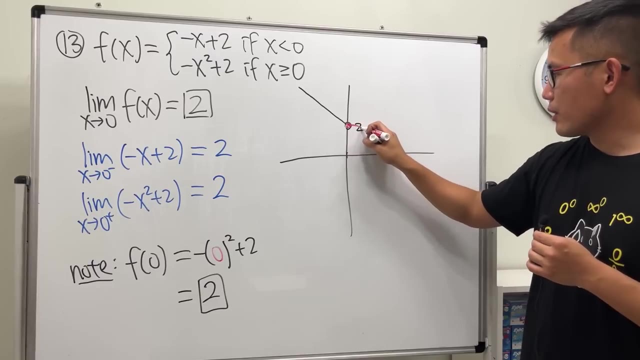 down parabola. however, it's been shipped up two units. it happens to be here and just the right hand side, because that's only when we have x is greater than equal to zero. so we started right here because thanks to equality here and then we have a parabola. so this right here is the line. 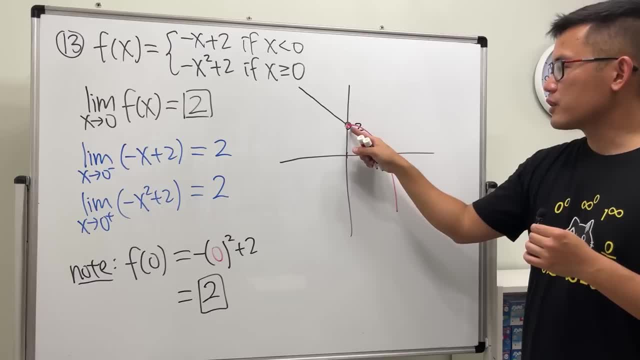 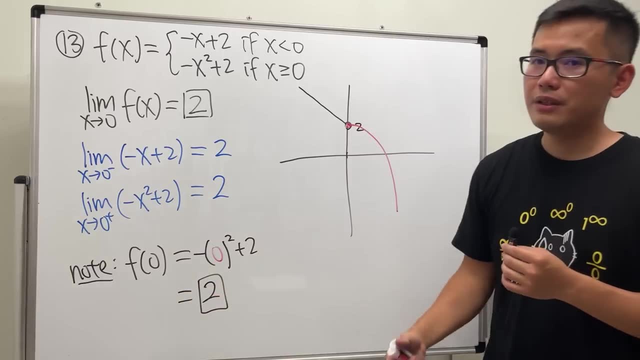 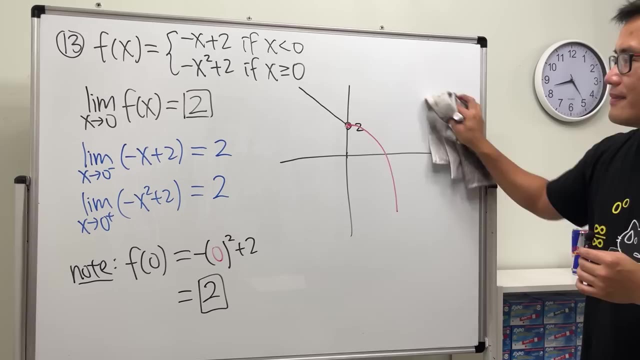 this right here is the parabola, and you can see that the function is continuous when x is equal to zero. that's why the limit and the value of the function: they are both equal to two because the function is continuous. all right. so hopefully this right here makes the piecewise function. 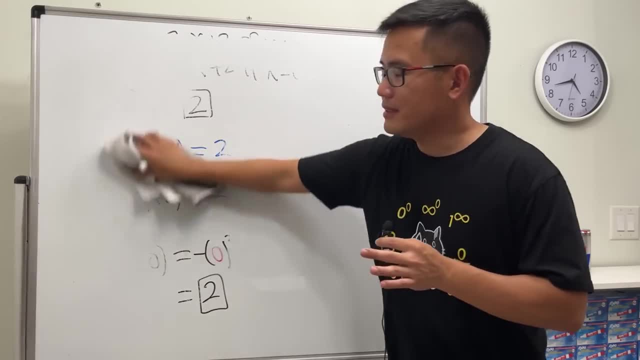 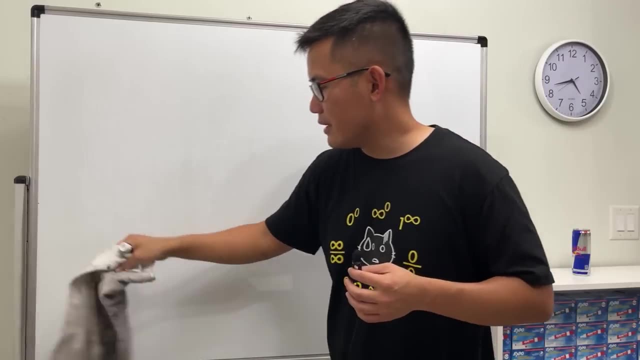 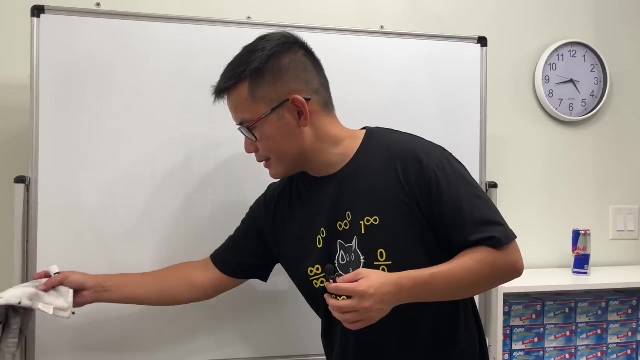 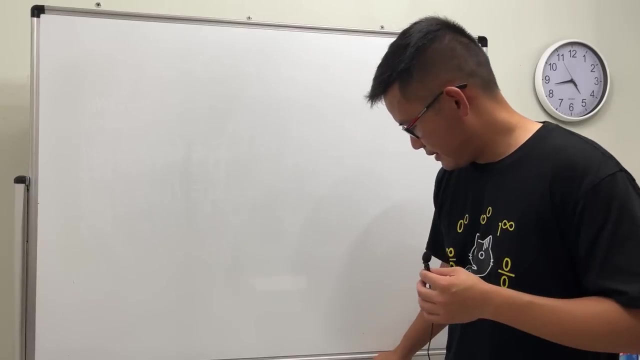 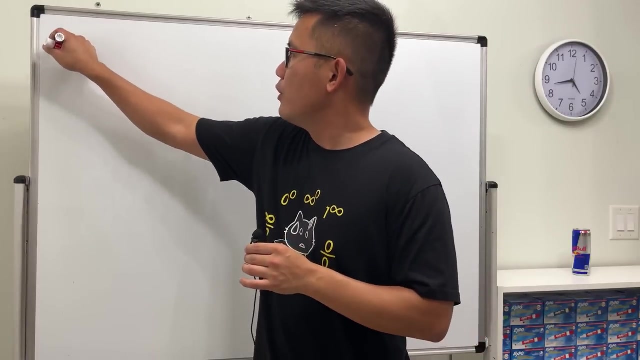 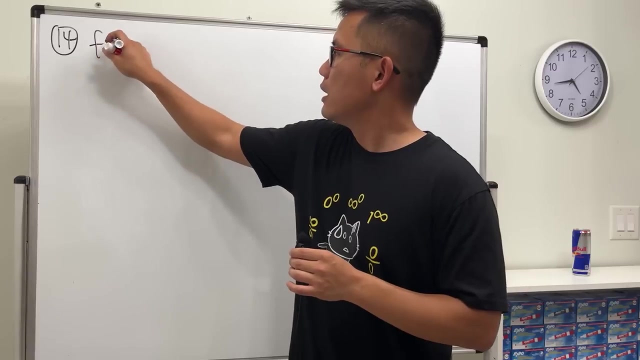 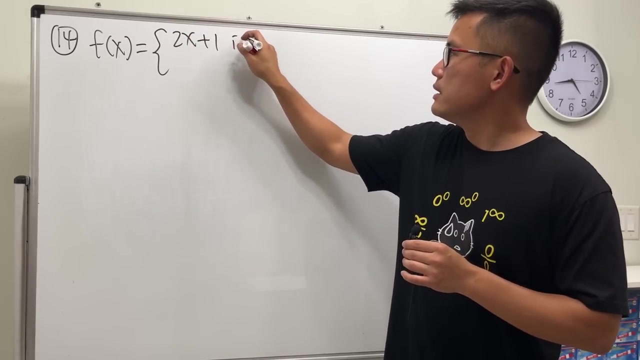 not so intimidating, because in fact you just really have to follow the direction like the condition, and then you do the piece here and there. that's all right. so so, and here's the solution. alright, number 14. our function is this: 2x plus one, and this is if x is greater than zero. 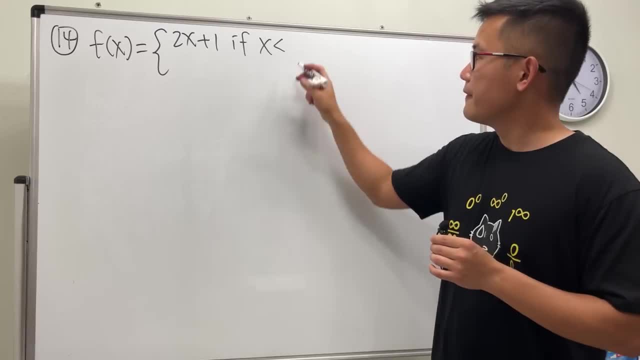 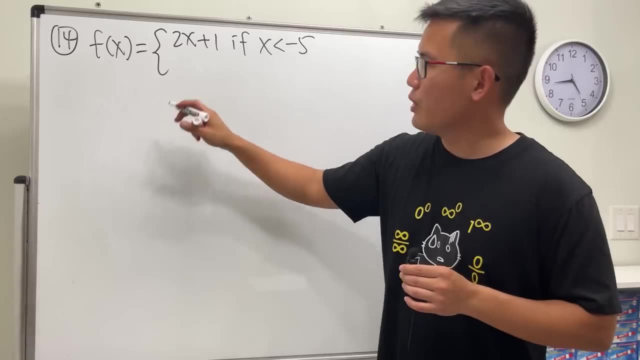 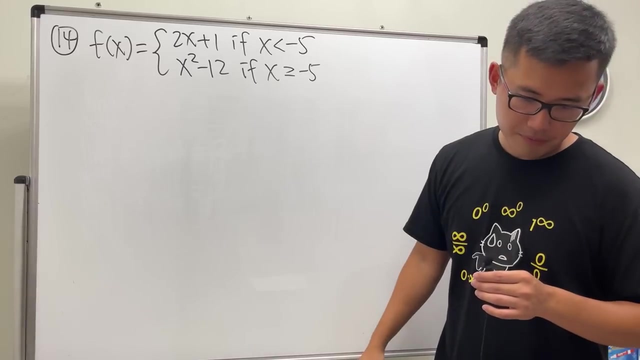 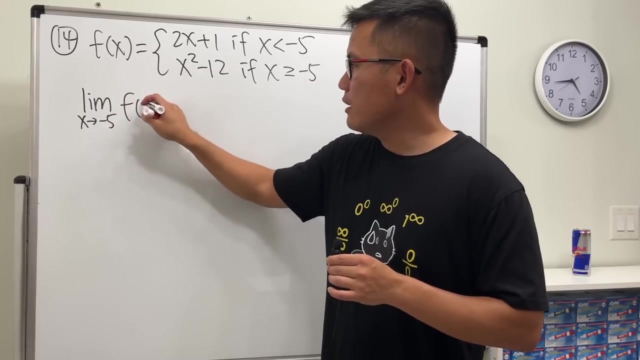 is less than negative 5, and then the other one is X square minus 12. this is, if X is greater than or equal to negative 5. all right, and you can guess it. the question is the limit as X approaching negative 5, of this function. okay, because 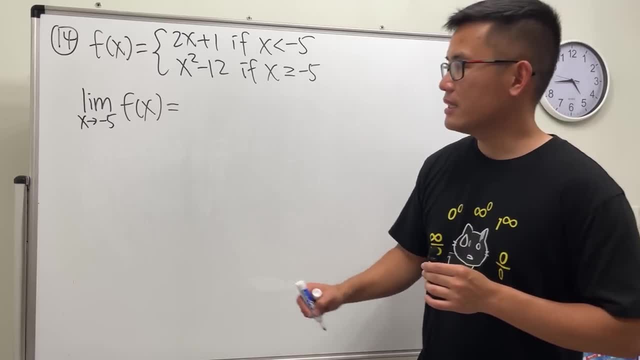 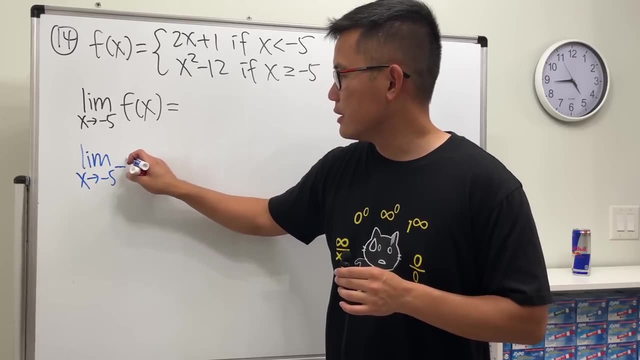 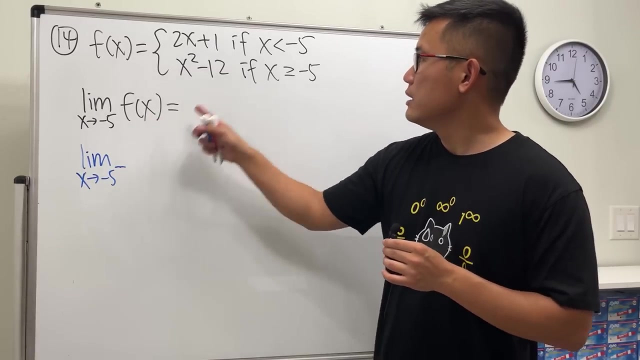 of the inequality that we have. so we do the left and right, yeah. so firstly, let's look at the limit as X approaching negative 5 on the negative side. so if X is approaching negative 5 on the left hand side or from the negative side, it's. 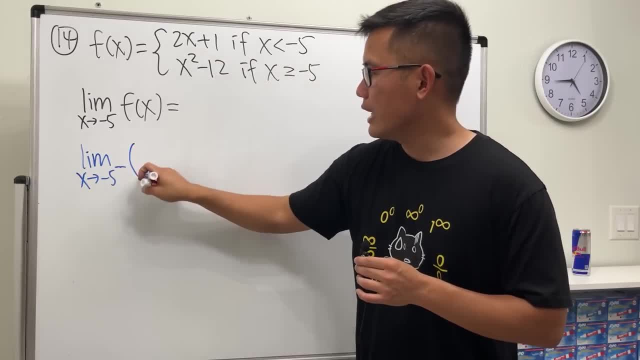 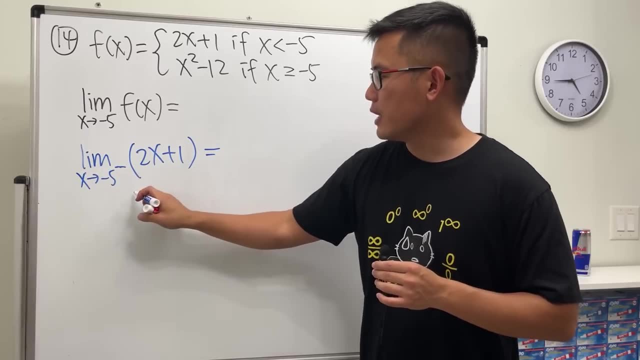 less than negative 5. so that means we look at this piece. so we have 2x plus 1. how do we do this? well, just plug in negative 5 in here and we get 2 times negative 5, and then we get negative 5, and then we get negative 5, and then we get. 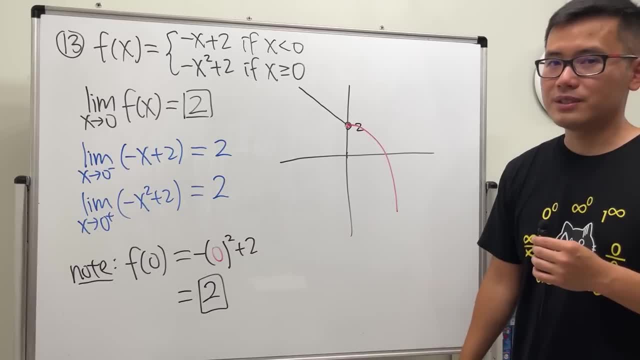 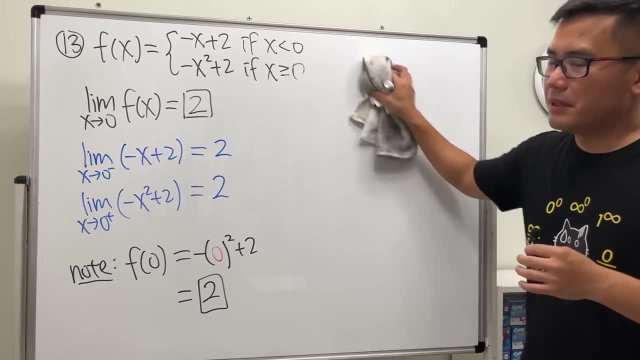 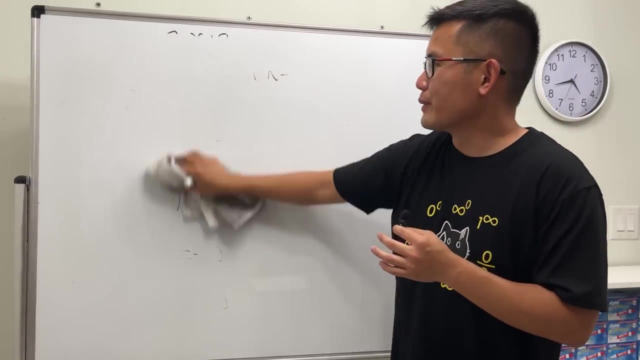 the function. they are both equal to 2, because the function is continuous, Alright, Okay. So hopefully this right here makes the piecewise function not so intimidating, because in fact you just really have to follow the direction, like the condition, and then you 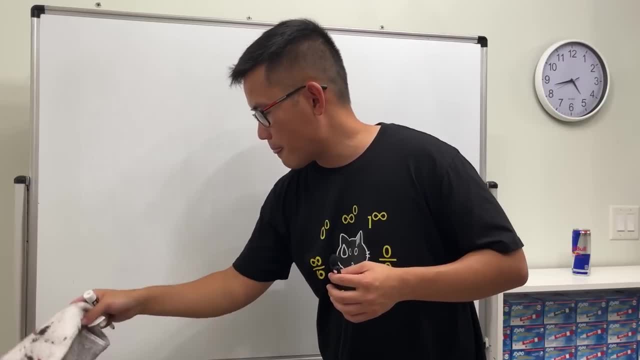 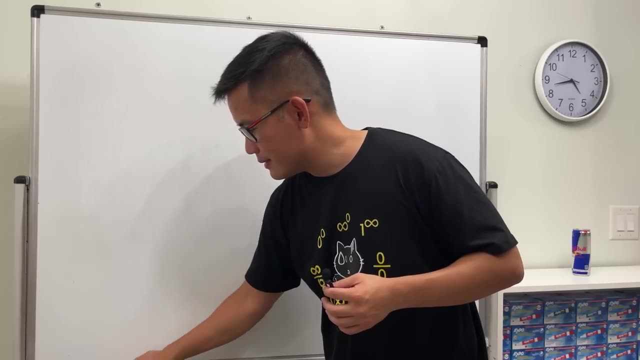 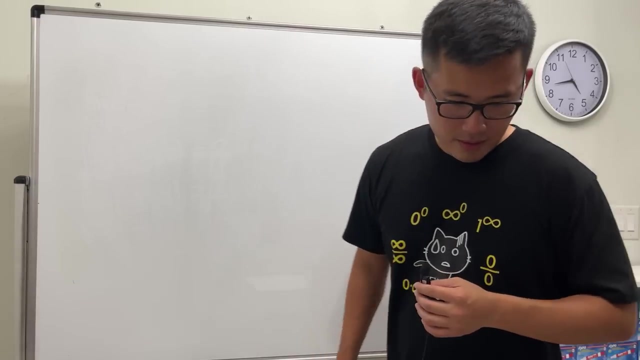 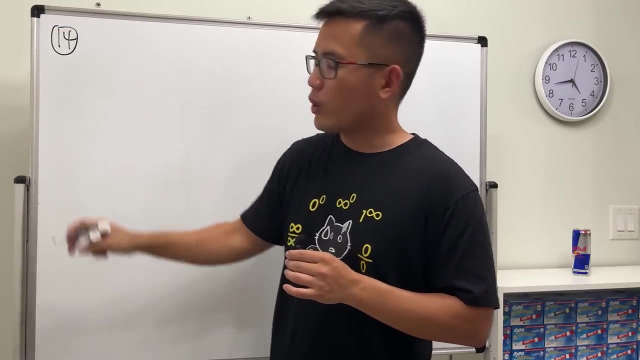 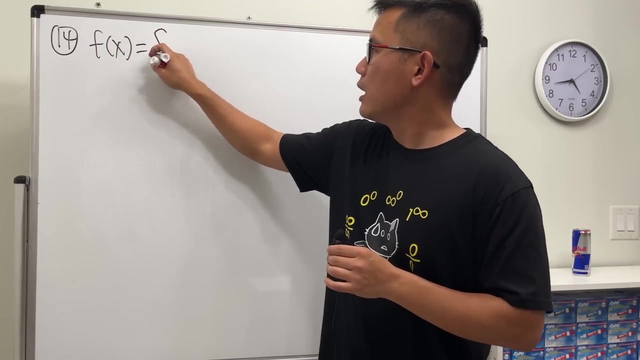 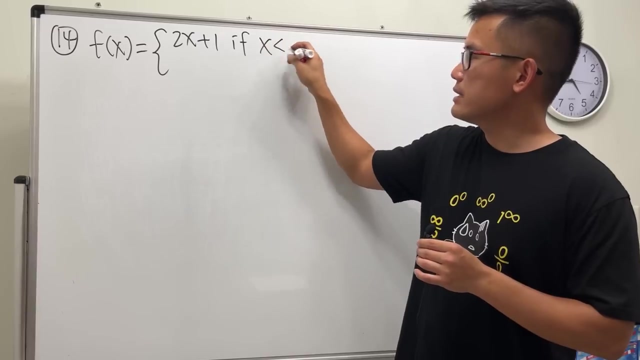 do the piece here and there. that's all Alright. number 14 of function is this: 2x plus 1, and this is if x is less than negative 5.. And then the other one is x squared- Alright. 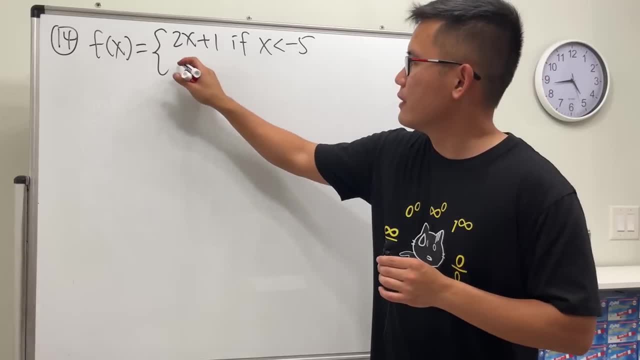 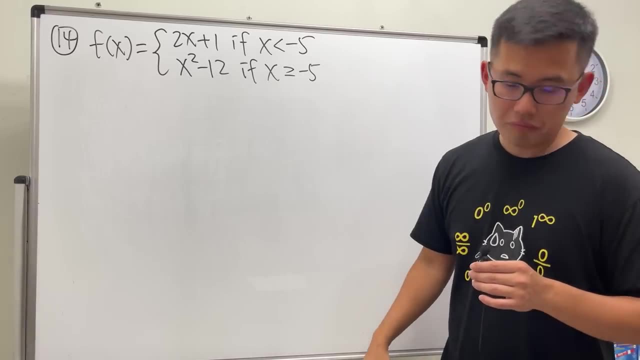 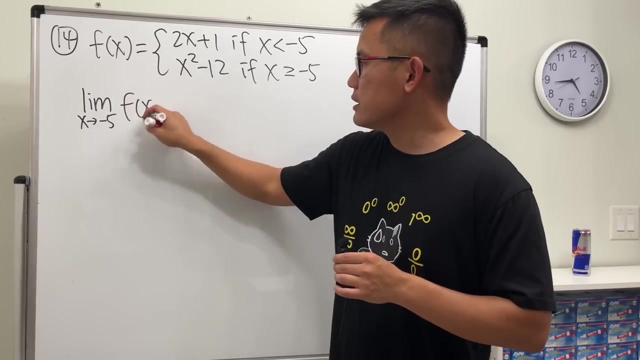 Okay, So if x is greater than or equal to negative 5,, this is, if x is greater than or equal to negative 5.. Alright, and you can guess it. the question is the limit as x approaching negative 5 of this function. 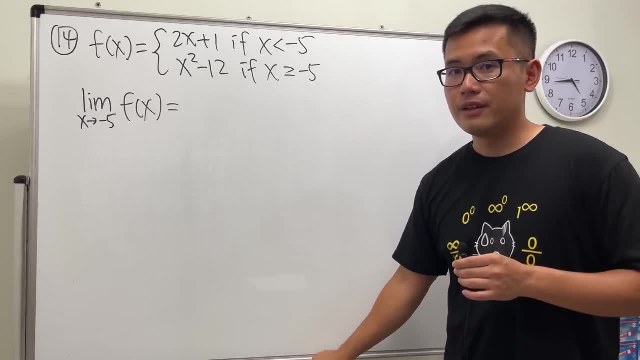 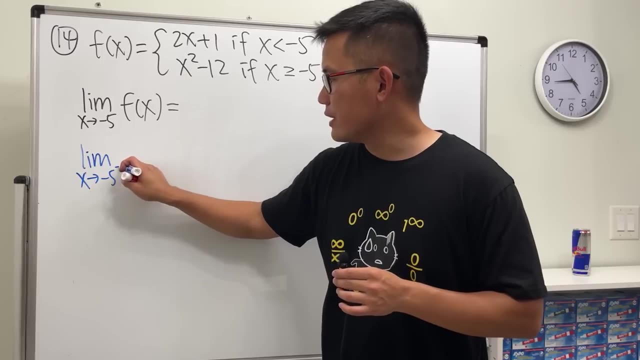 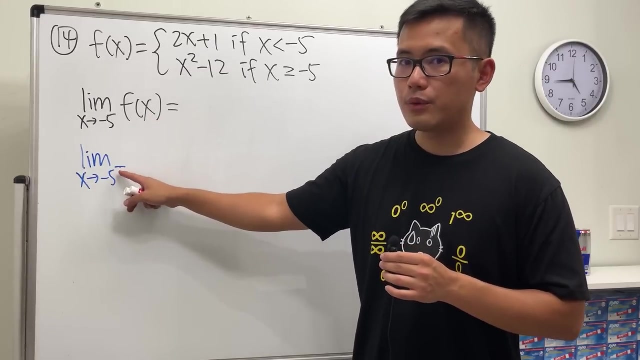 Okay, Because of the inequality that we have, so we do the left and right, yeah. So, firstly, let's look at the limit as x approaching negative 5 from the negative side. So if x is approaching negative 5 from the left-hand side or from the negative side, 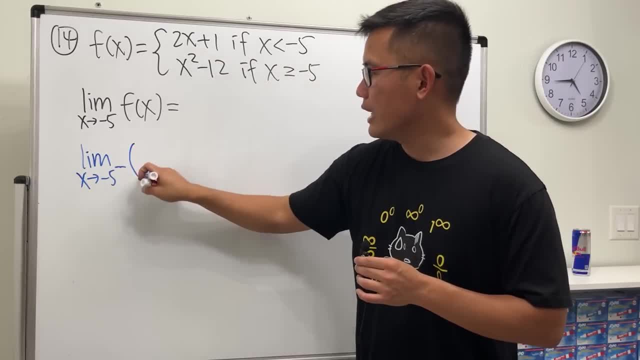 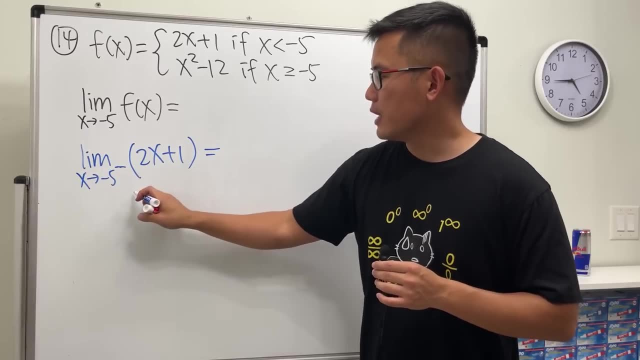 it's less than negative 5, so that means we look at this piece, so we have 2x plus 1.. How do we do this? Well, just plug in negative 5 in here and we get 2 times negative 5 plus 1, and that's. 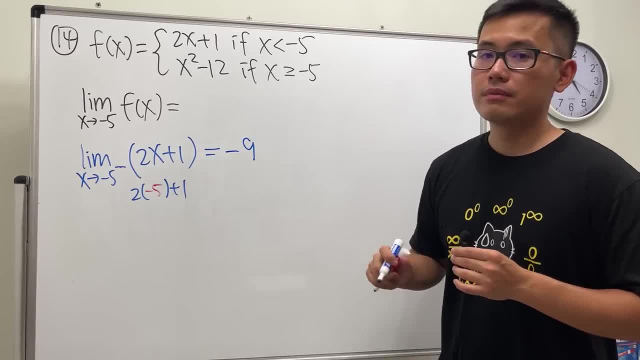 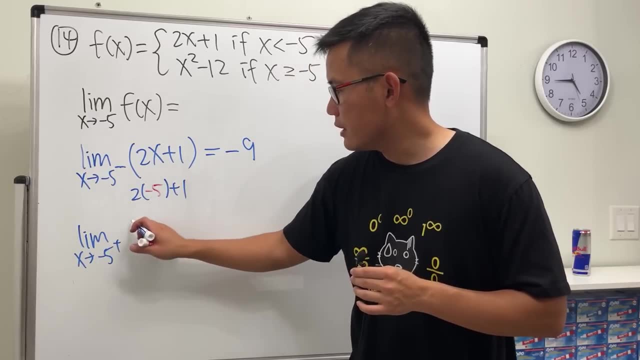 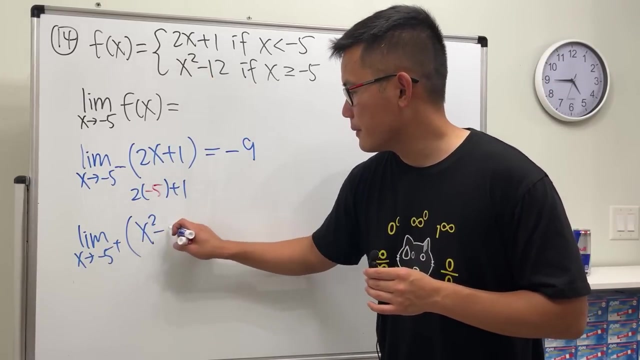 negative 10 plus 1, which is negative 9.. Okay, On the other hand, When we have the limit as x approaching negative 5, positive, that means we do this right, Which is x squared minus 12. And to do so, just plug in negative 5 in here and just work that out. 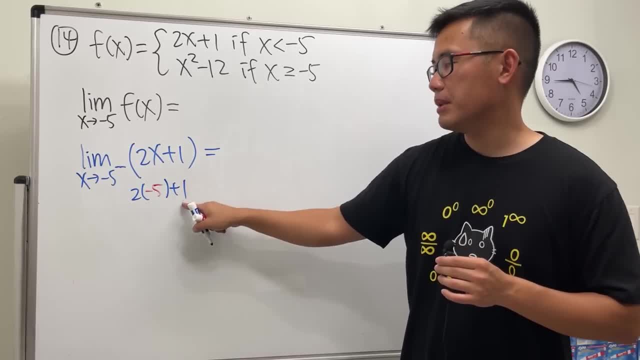 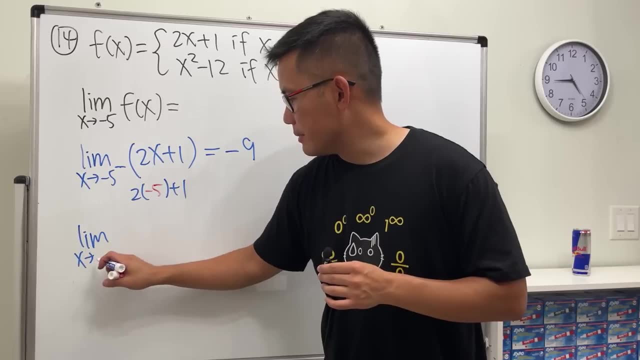 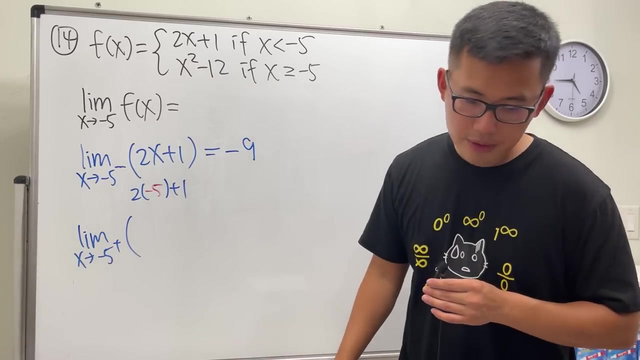 negative 5 plus 1, and that's negative 10 plus 1, which is negative, 9, okay. on the other hand, when we have the limit as X approaching negative, 5 positive, that means we do this right, which is X square minus 12, and to do so, just plug in. 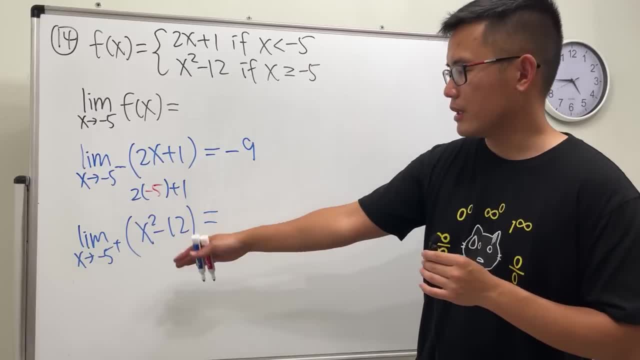 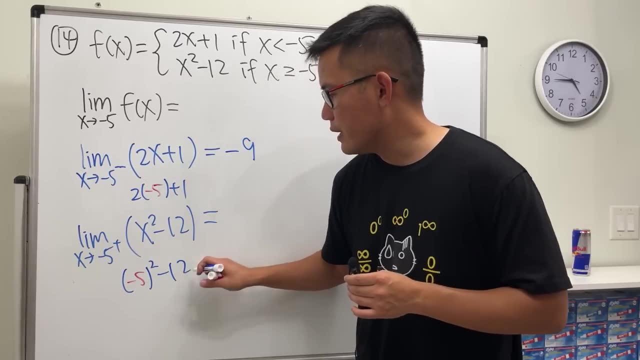 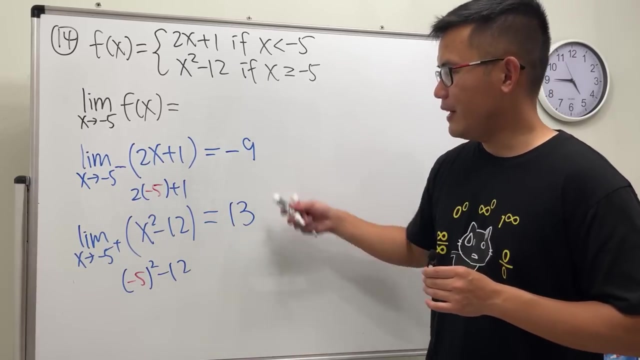 negative 5 in here and just work that out, because this is not like we're in determinate form. so just plug in, work out. that would be the answer. so negative 5 square minus 12, that's 25 minus 12, 13 very different so. 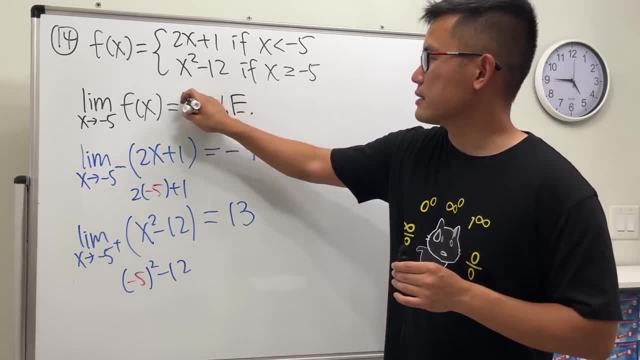 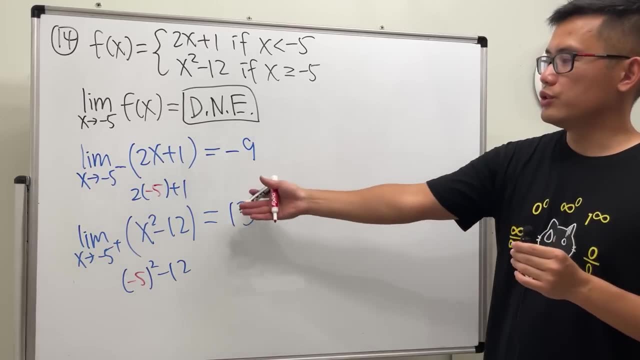 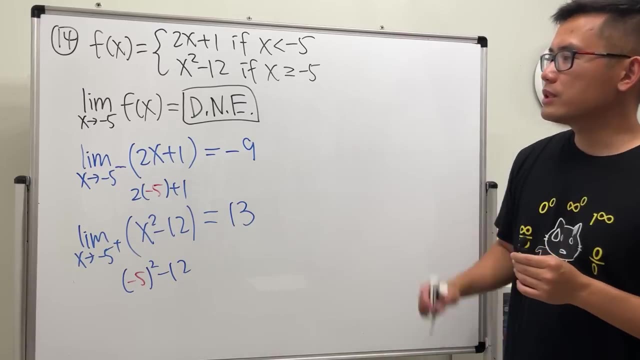 the answer is does not exist. you see, if the question doesn't ask you to make graphs, then this right here will be it. just show this and that and then draw the conclusion for the limit as X approaching negative 5. but of course I'll give you guys the graph real quick, just to make things super, super clear, because 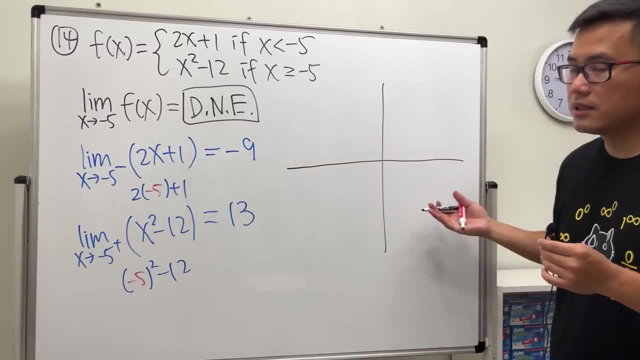 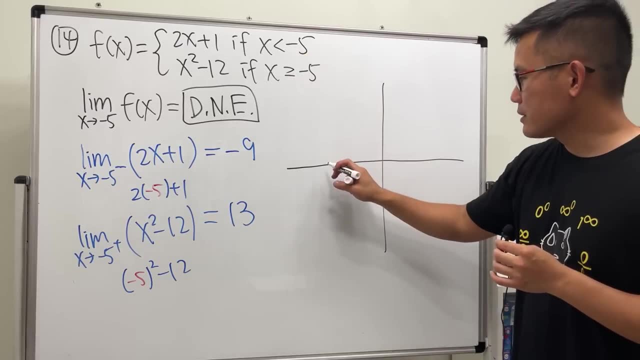 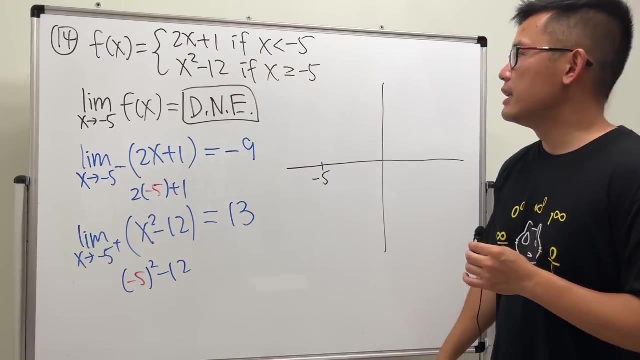 this is for practice, right? if I on the test, if they just wants to figure the answer, I will stop right there. okay, we care about negative Phi. that says right here this: it's a line with positive slope and let's see, when X is negative Phi, we get negative 9. so we should have negative Phi and negative 9. 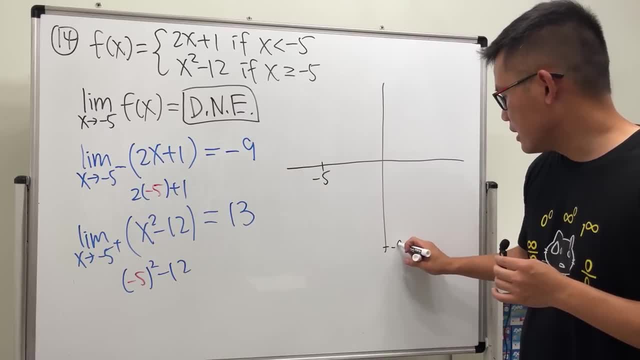 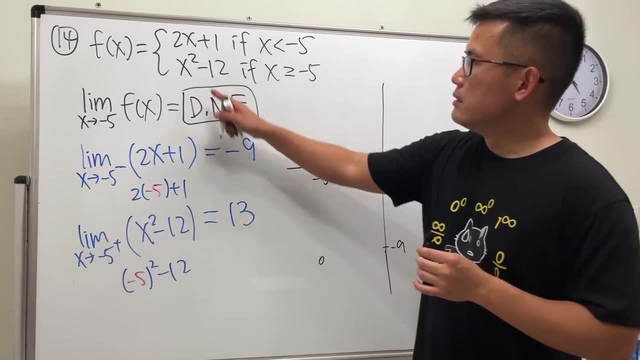 we get negative 9, so we should have negative Phi, and negative 9, so we should have negative Phi, and also let's say this is negative nine, and then we have an open circle like so okay, and then uh, two, so you should have a positive slope. so the picture should look like this: 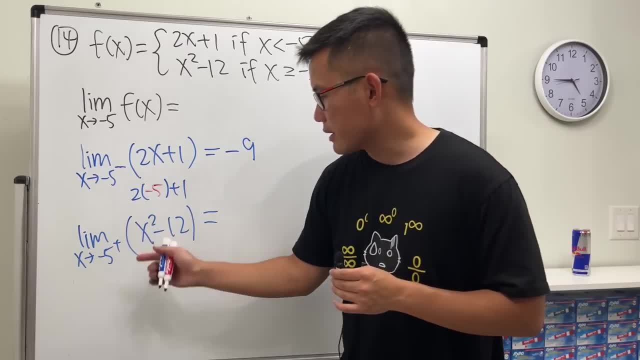 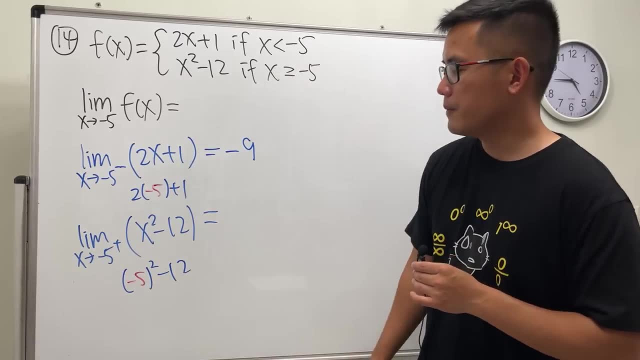 Because this is not like weird, like indeterminate form, so just plug in, work it out, that will be the answer. So negative 5 squared minus 12. That's 25 minus 12. 13. Ah, Very different. 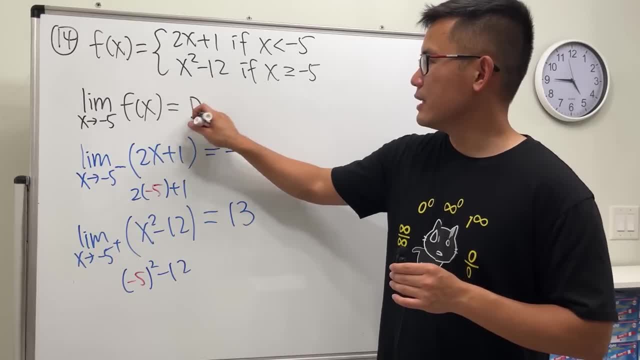 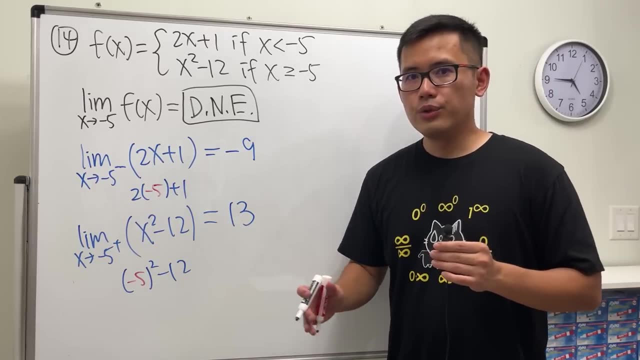 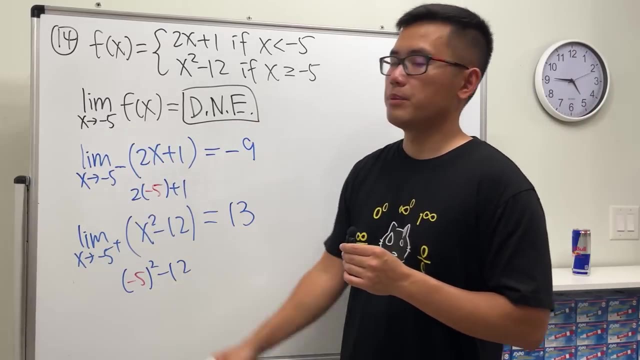 So the answer is does not exist. You see, if the question doesn't ask you to make graphs, then this right here will be it. Just show this and that and then draw the conclusion for the limit as x approaching negative 5.. 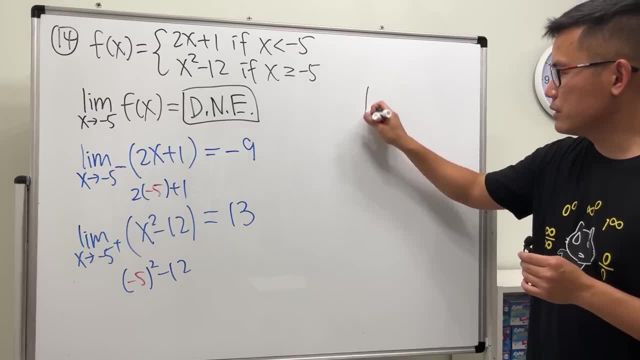 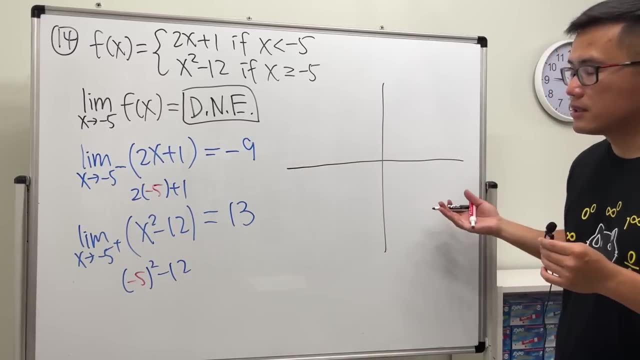 But of course I'll give you guys the graph real quick just to make things super, super clear, Because this is Focus, Focus, Focus, Focus, Focus, Focus Focus. Okay, So we just have to practice, right. 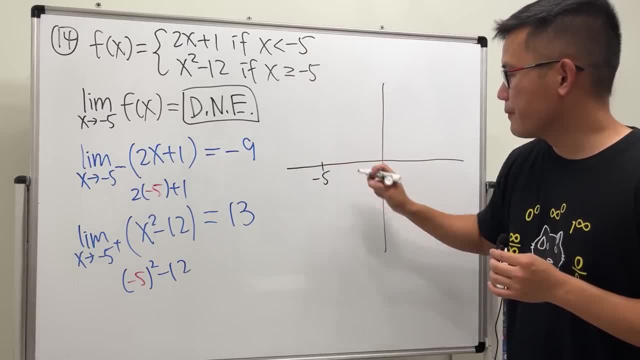 If you are on the test. If they just want us to figure out the answer, I will stop right there. Okay, We care about negative 5. that says, right here, This is a line which is positive slope, And Let's see. 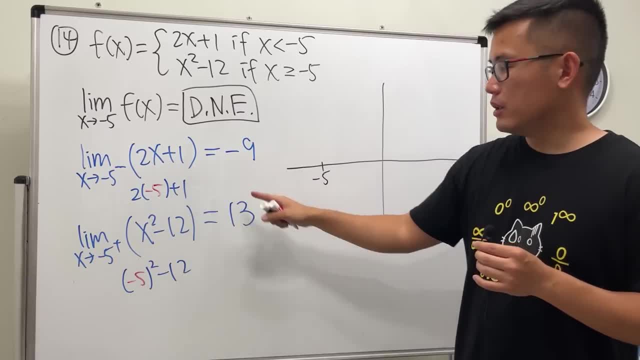 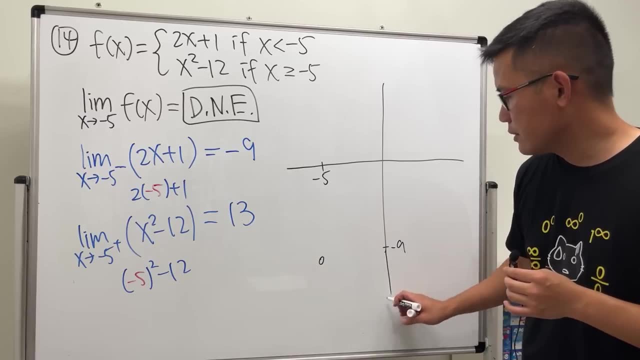 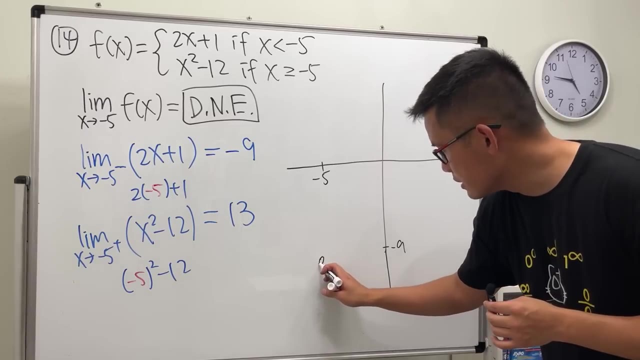 When x is a negative 5, we get negative 9.. So we should have negative 5 and also let's say this is negative 9.. And then we have an open circle like so Okay, And then 2, so you should have a positive slope. so the picture should look like this: slope 2,. 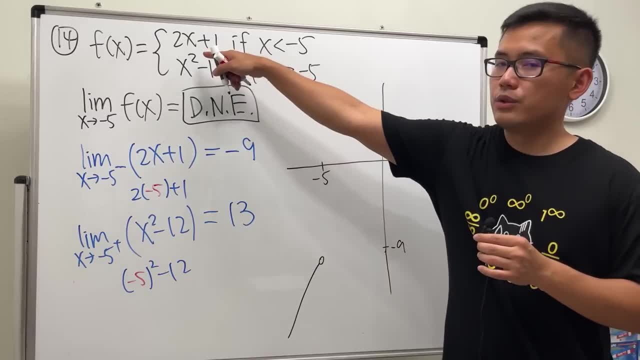 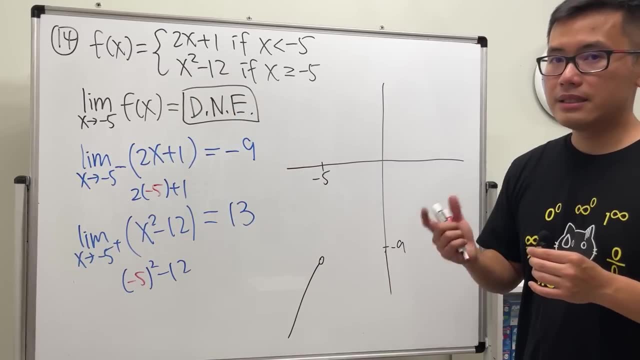 or, if you would like, you can just plug in, let's say negative 6, and then plug into: there, work that out. yeah, that's okay. what's this? this is a parabola. yeah, this is a. 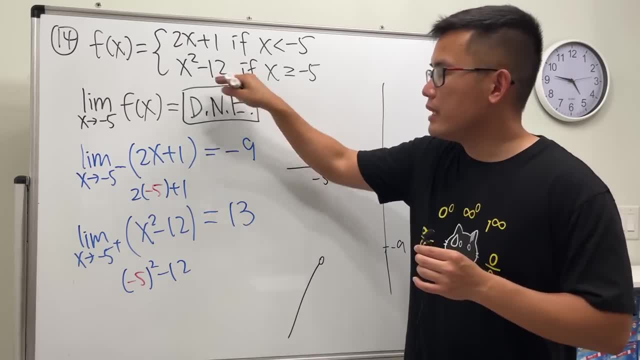 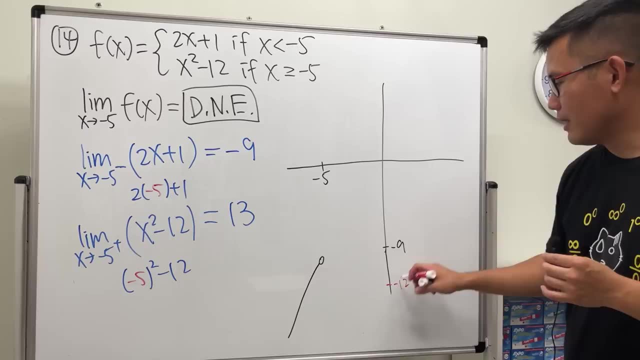 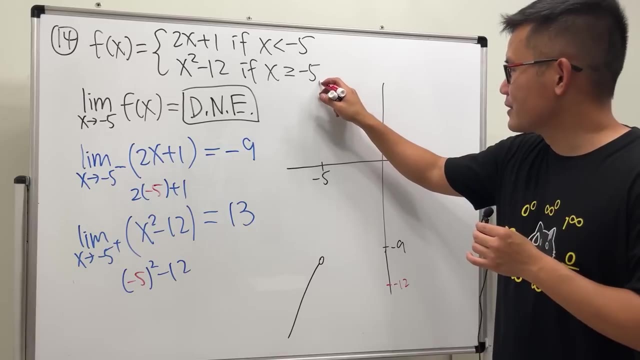 parabola x squared, but you drag it down 12 units. so let's say this: right here is negative 12, and then you just have a parabola that looks like this: but when x is a negative 5,, the value is 13,. so the picture is going to look like this. it's crazy, it's symmetric. 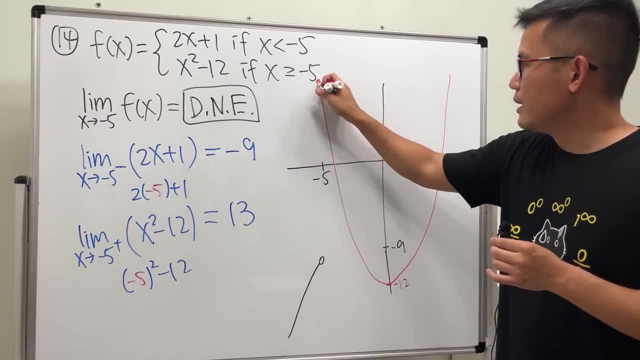 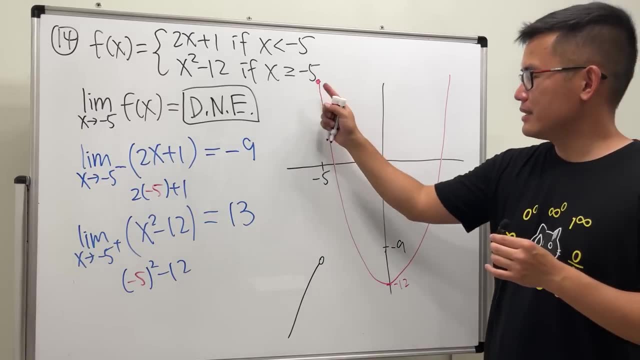 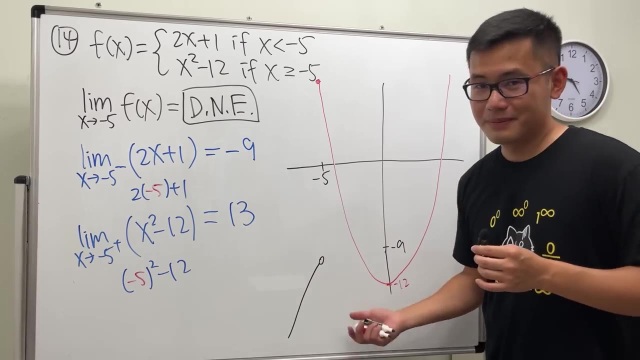 so I'll try my best. yeah, so this is the part that we were talking about: here we get negative 9, and then here we get a positive 13, that's it, Okay, And that's how you do it, yeah. 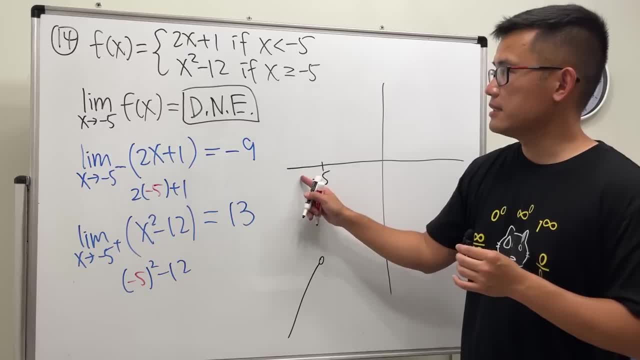 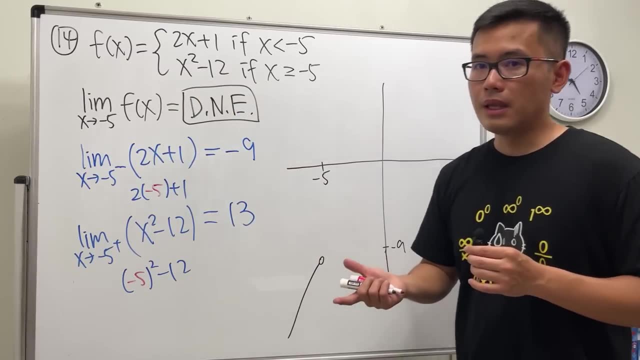 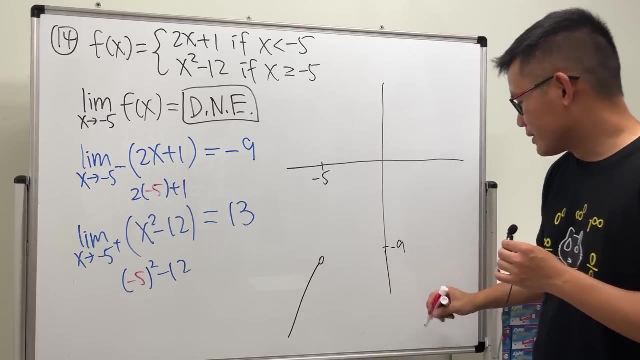 and slope two. or, if you would like, you can just plug in: let's say negative six and then plug into there. work that out. yeah, that's okay. what's this? this is a parabola. yeah, this is the parabola x squared, but you drag it down 12 units. so let's say this: right, here is negative 12. 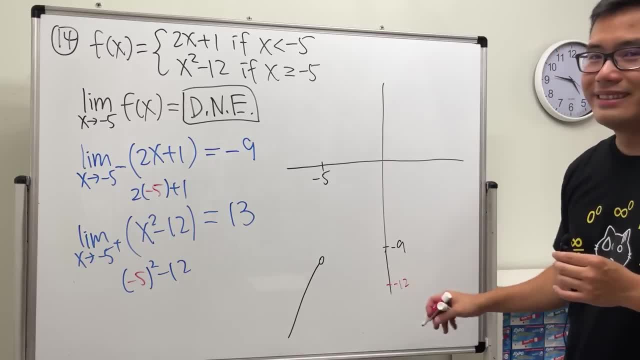 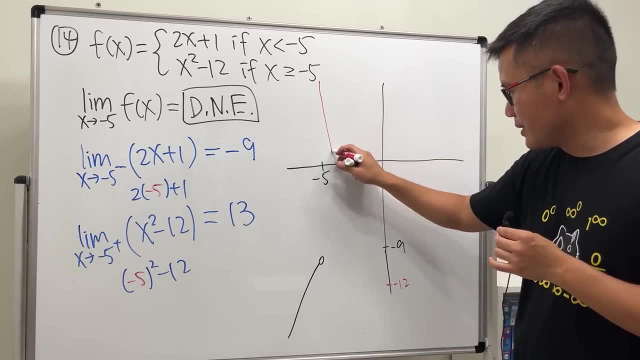 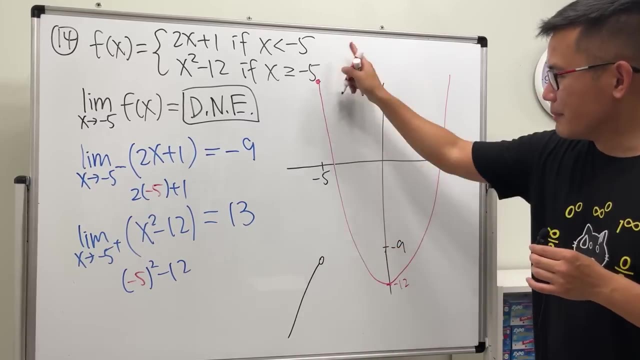 and then you just have a parabola that looks like this: but when x is at negative 5, the value is 13, so the picture is going to look like this. it's crazy, it's symmetric, so i'll try my best. so this is the part that we were talking about here. we get negative 9, and then 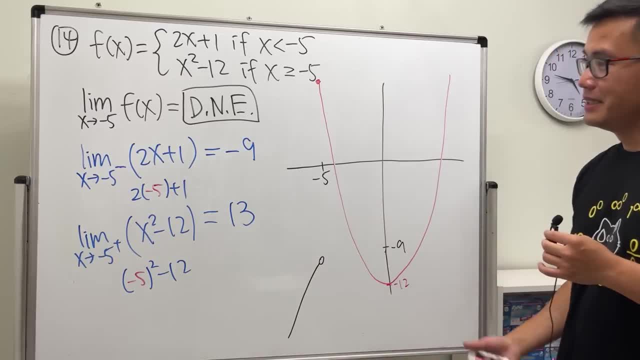 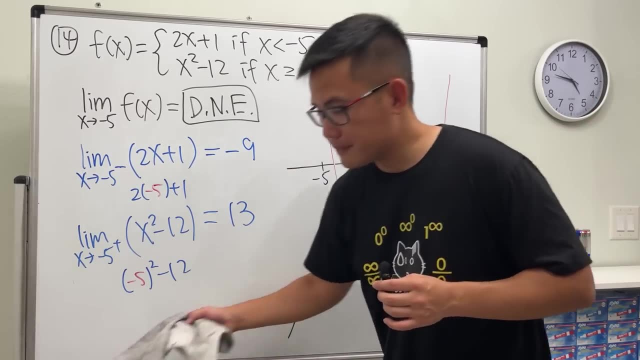 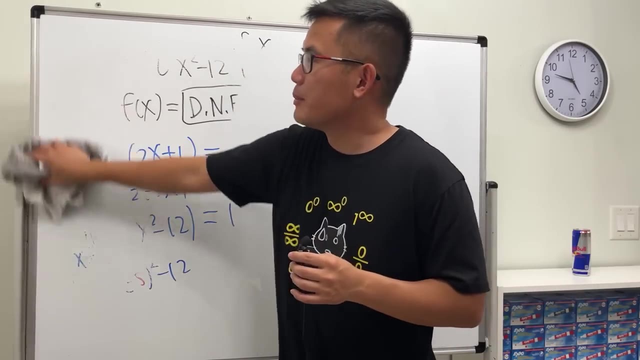 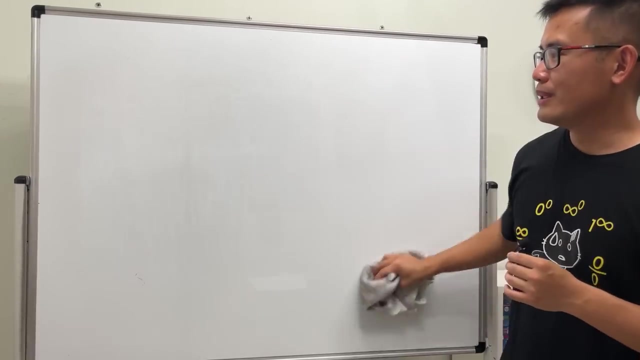 here we get a positive 13.. that's it and that's how you do it. yeah, okay, how are you guys doing? how are you guys doing? hopefully you guys are doing good, you know. just a couple more questions to go right. hang there. if i can do it, you guys can do it too. you don't have to watch this video one time through, right. 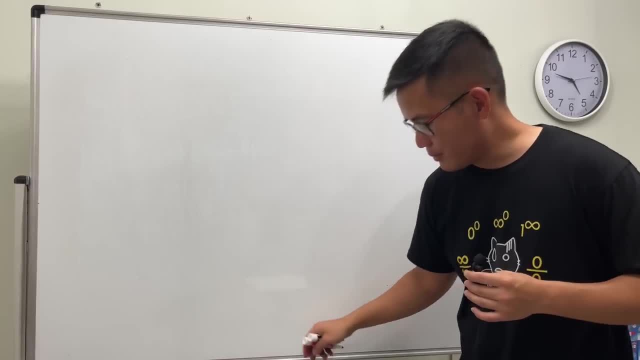 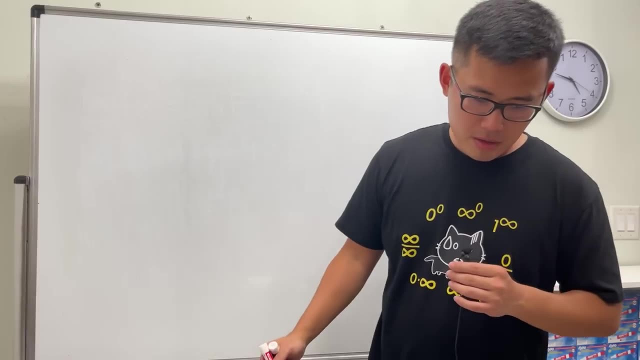 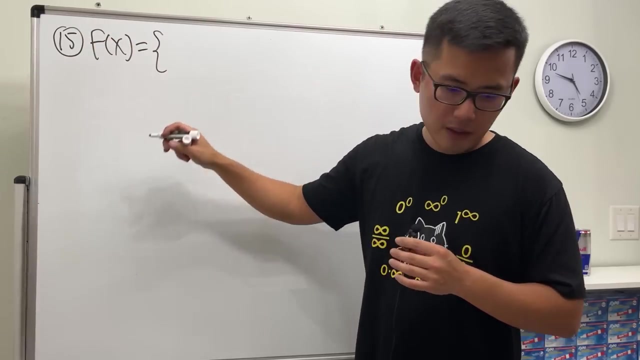 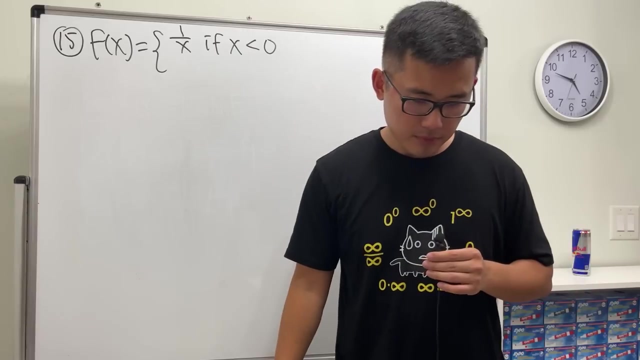 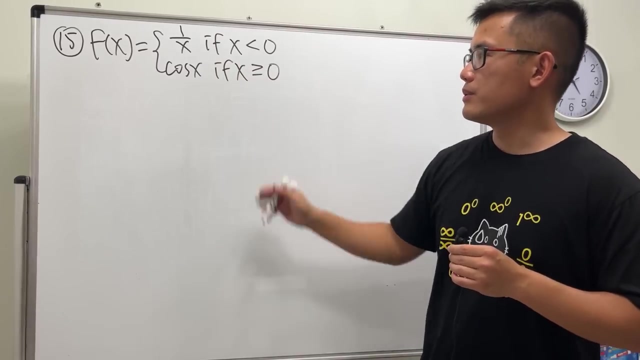 break if you would like, but just make sure that you do the practice all right. number 15, function f of x equals: first, we have 1 over x. if x is less than 0, if x is greater than 0, we get cosine x also including 0. yeah, so let's see. 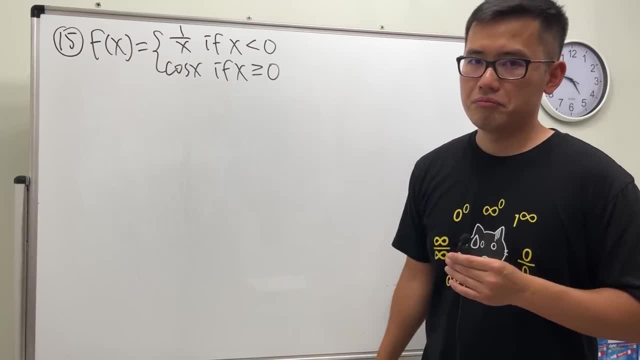 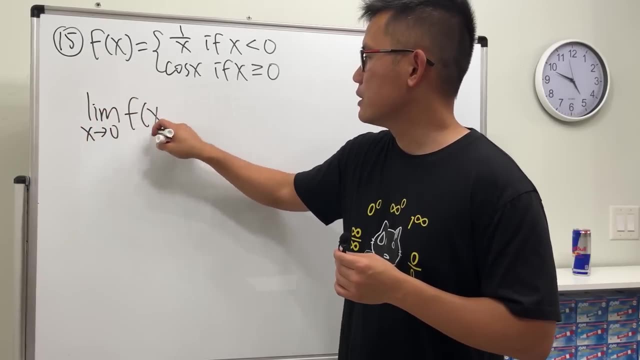 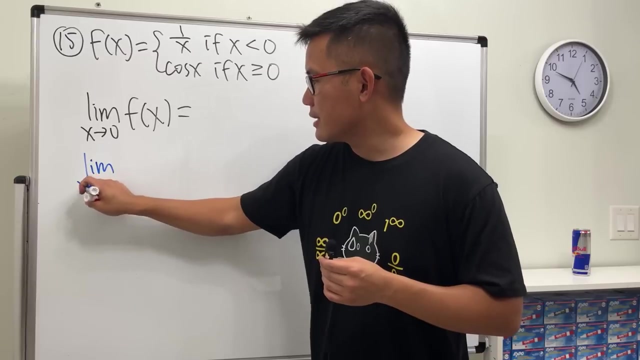 i think for this one let's just do the graph and then find the answer. so if we want the limit as x approaching 0 of the function again, we will have to do a left and right. let's still do 11, right? so firstly we do the limit as x approaching 0 minus. if it's 0 minus, then the function that we 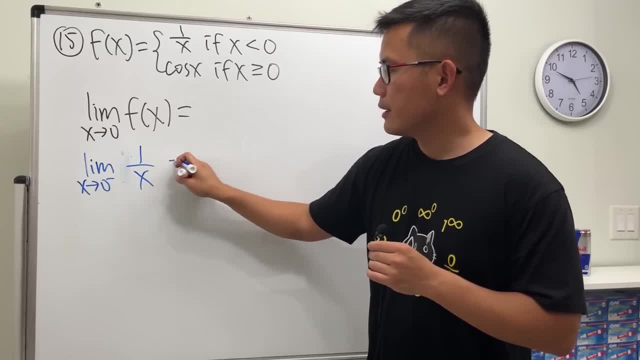 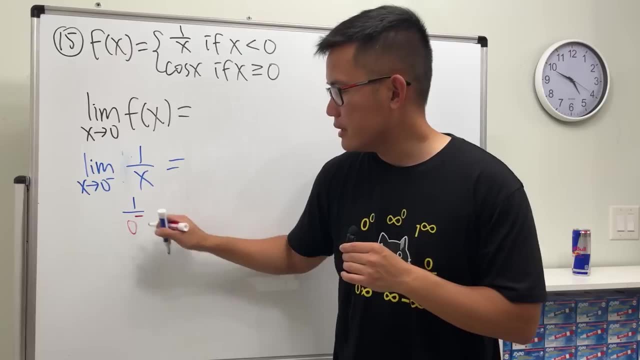 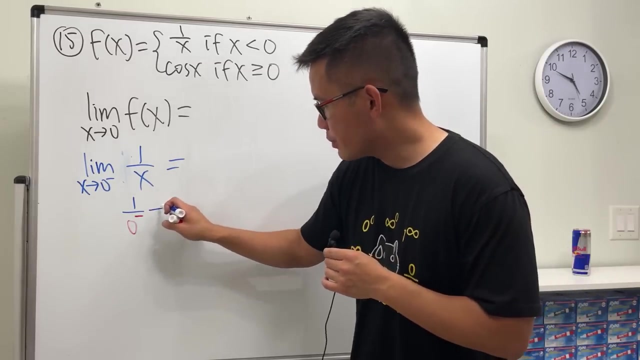 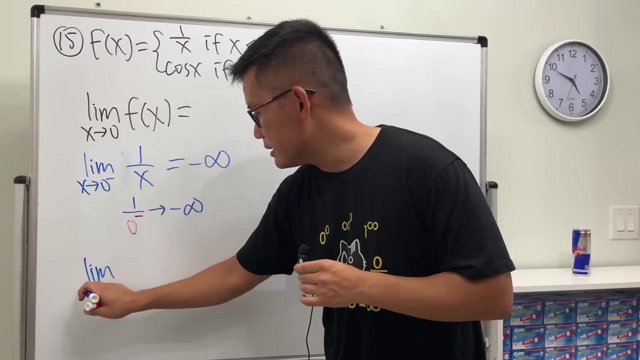 need to use is 1 over x. so what's the answer for this, though? well, we put 0 minus in here. we get 1 over 0 minus positive divided by negative, and then we have a 0 right limit, 4 on the bottom. so this right here approaches negative infinity, and if we have the limit as 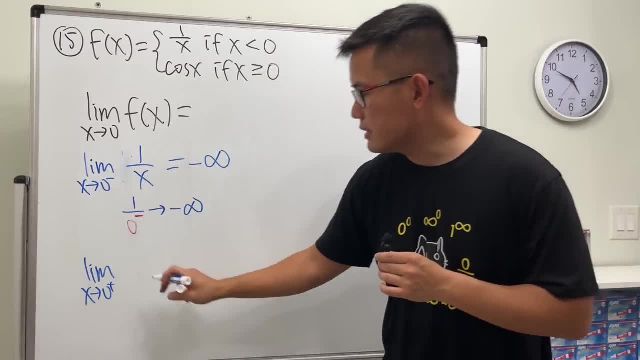 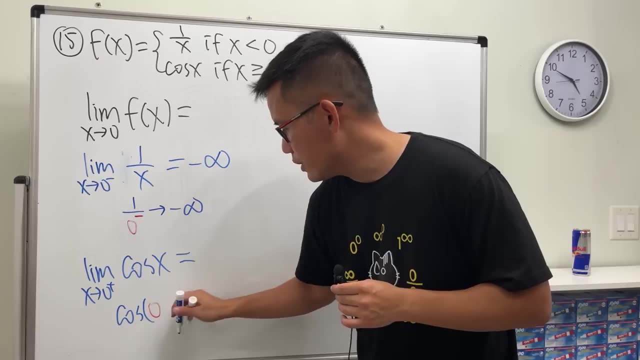 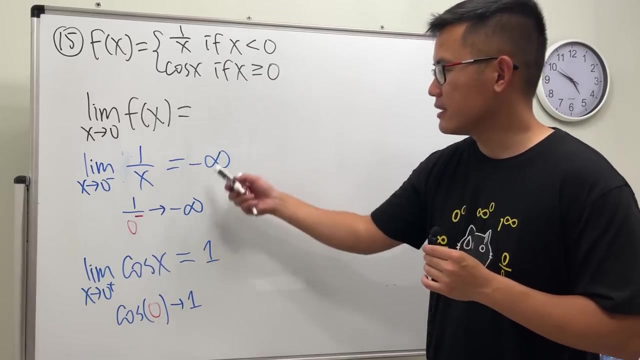 x approaching 0. plus we look at cosine x and for this right here, just plug in 0 into cosine and then we can actually work that out and we get 1 right. so the answer is just one: cool, but the thing is that they are not equal. therefore, 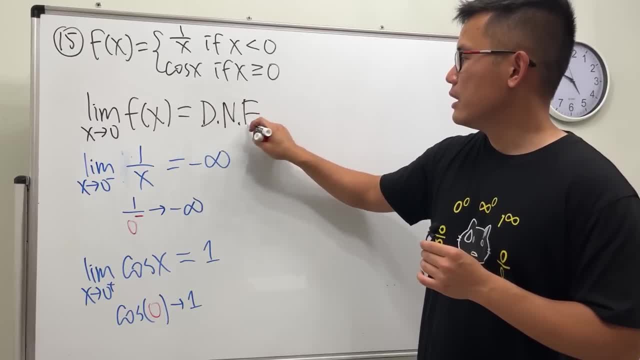 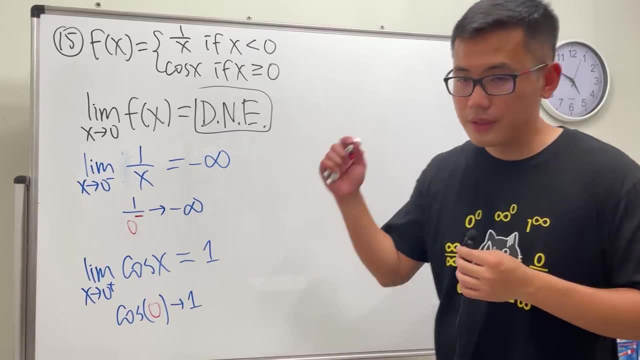 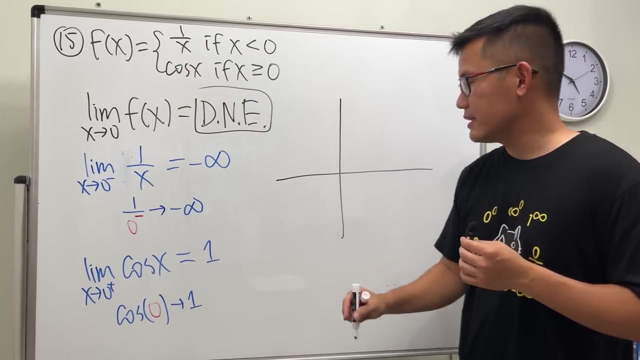 the answer right here does not exist. it does not exist, okay. and then, oh, let me make you guys a crap real quick, for if less than zero, we do one over x, and 1 over x is greater than 0.. of x is like this: right, this is one of x. usually it's like this and that, but here we just care. 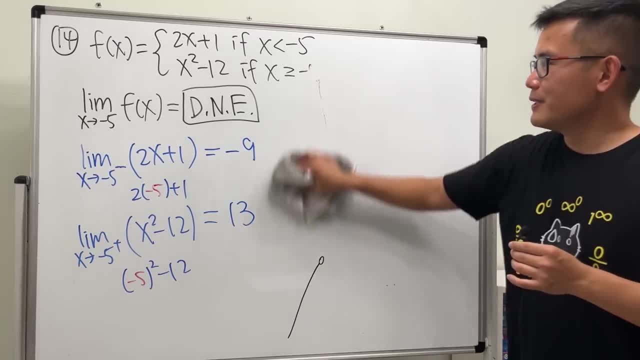 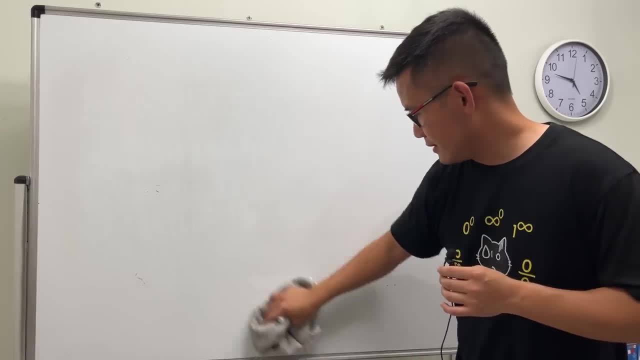 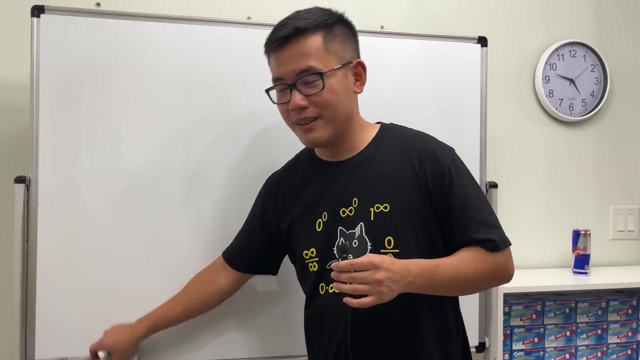 Okay, how are you guys doing? how are you guys doing? hopefully you guys are all doing good. just a couple more questions to go right. hang there. if I can do it, you guys can do it too. you don't have to watch this video one time through. right, take a break. 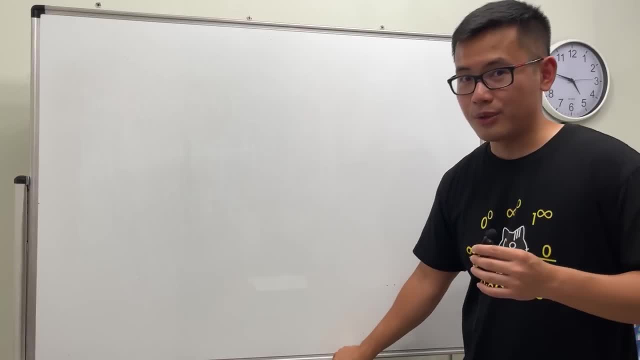 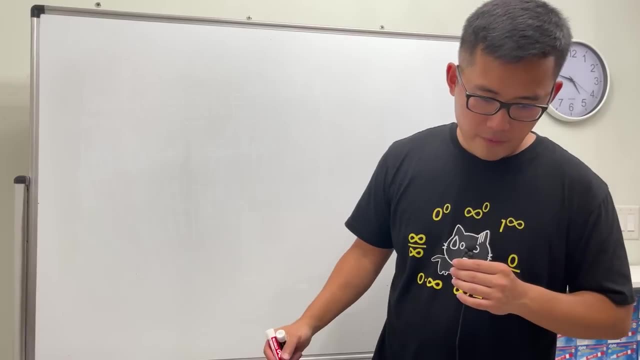 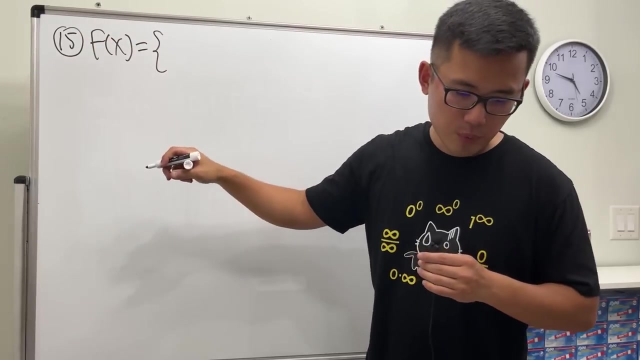 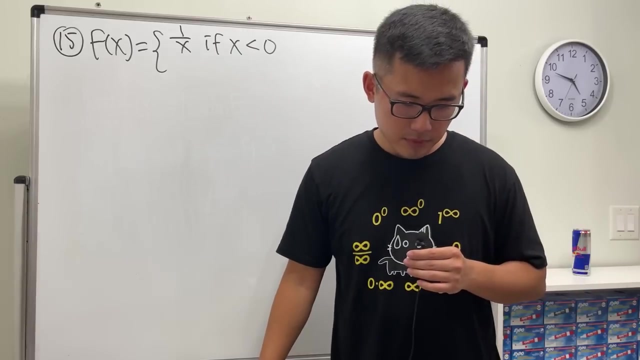 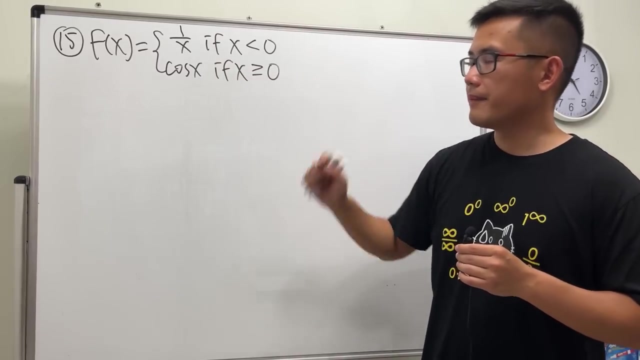 if you would like, but just make sure that you do the practice right. Number 15, function f of x equals: first, we have 1 over x if x is less than 0,. if x is greater than 0, we get cosine x, also including 0, yeah, so let's see. 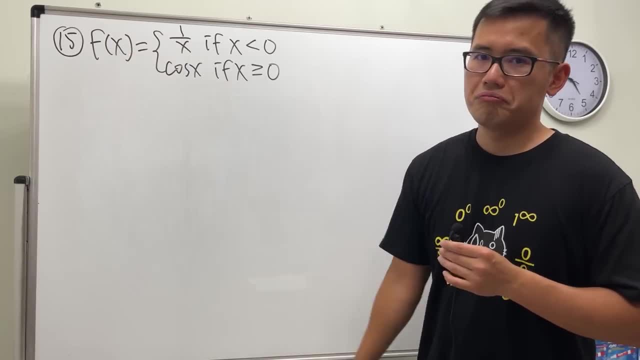 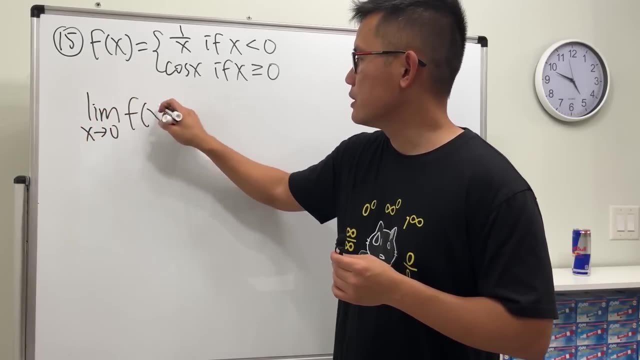 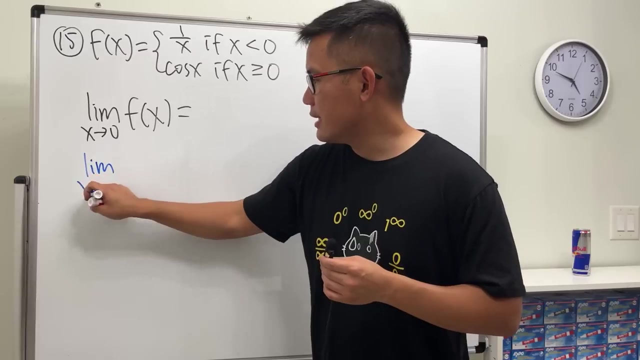 I think for this one let's just do the graph and then find the answer. so if we want the limit as x approaching 0 of the function again, we will have to do it left and right. let's still do it left and right. so firstly we do the limit as x approaching 0 minus. 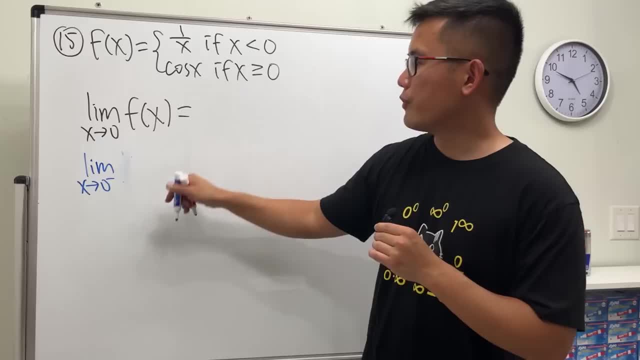 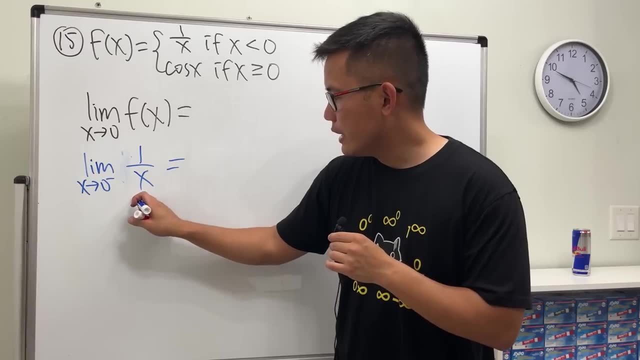 if it's 0 minus, then the function that we need to use is 1 over x. so what's the answer for this, though? Well, we put 0 minus In here. we get 1 over 0 minus positive, divided by negative, and then we have a 0, right. 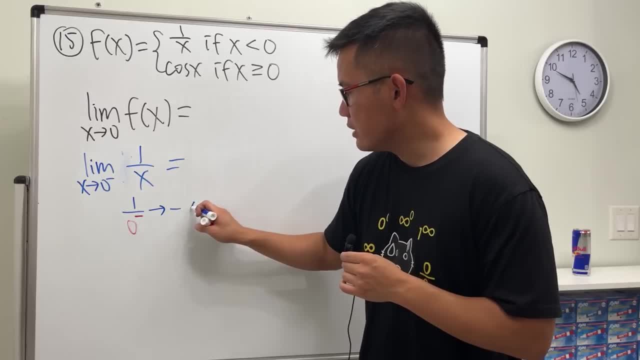 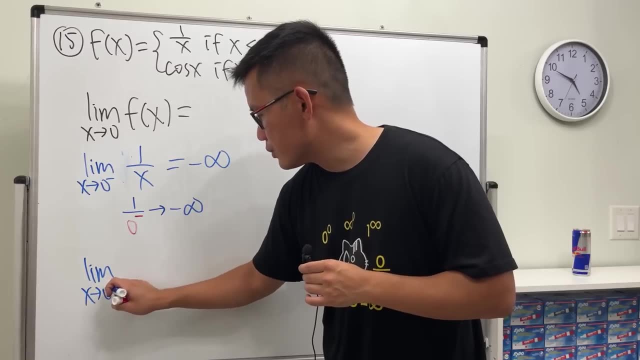 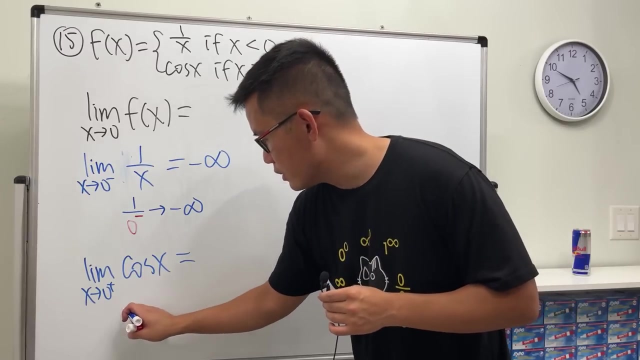 limit 4 on the bottom. so this right here approaches negative infinity. and if we have the limit as x approaching 0 plus, we look at cosine x and for this right here just plug in 0 into cosine and then we can actually work that out and we get 1.. 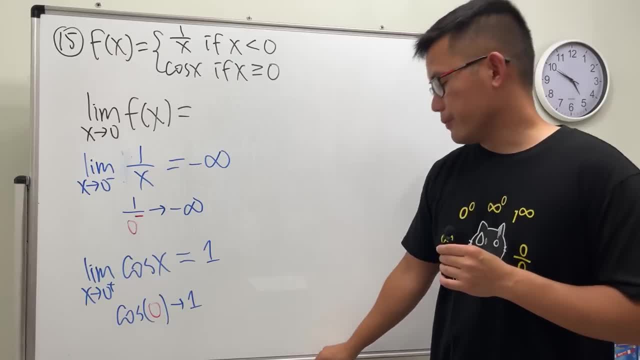 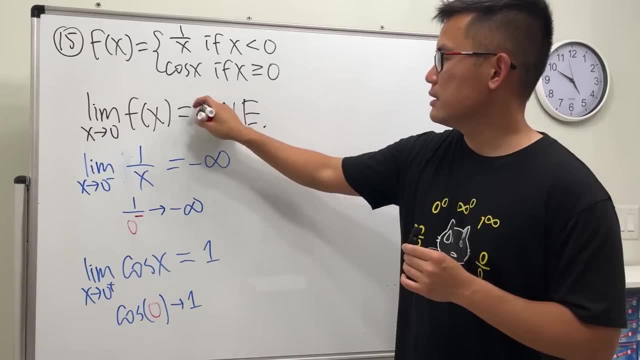 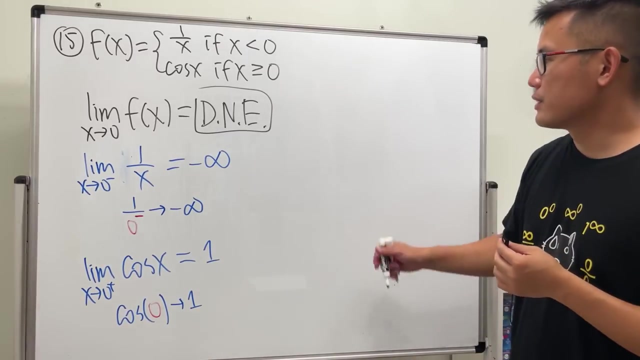 Right, so the answer is just 1,. cool, but the thing is that they are not equal. therefore, the answer right here does not exist. right, does not exist, okay. and then, oh, let me give you guys a graph real quick. when it's less than 0, we do 1 over x and 1 over x. 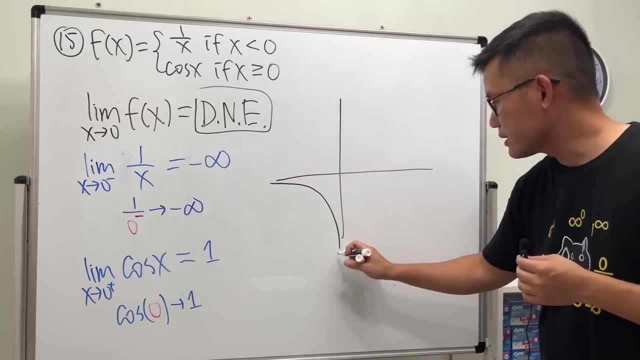 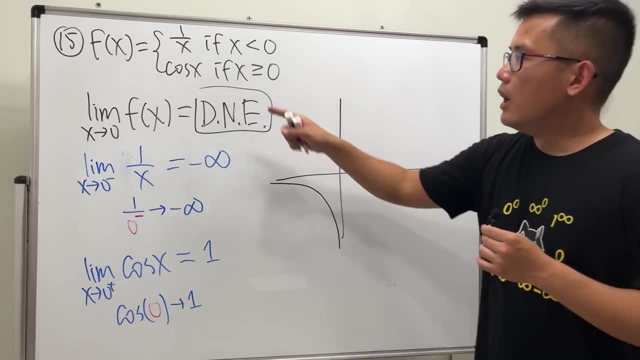 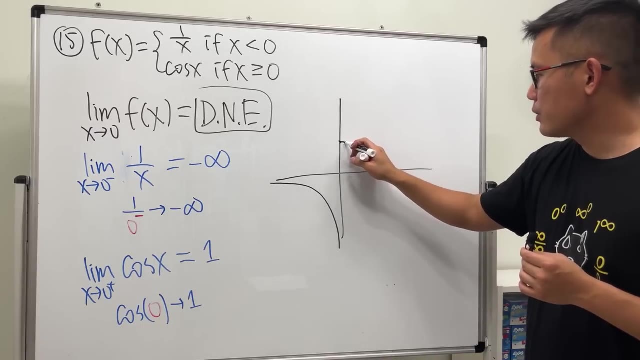 is like this: right, this is 1 over x. usually it's like this and that, But here we just care about when x is less than 0, so just this part: Cosine x. cosine starts with 0 comma 1, right, so we start right here, and then it goes down. 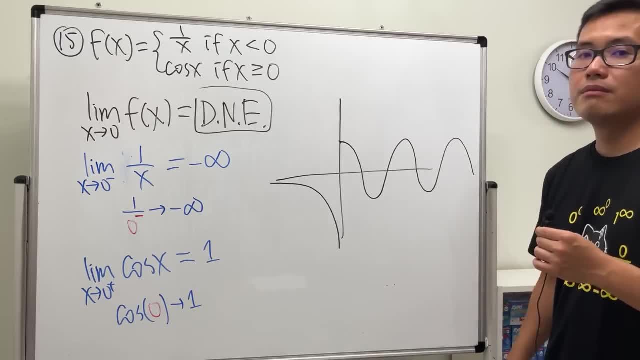 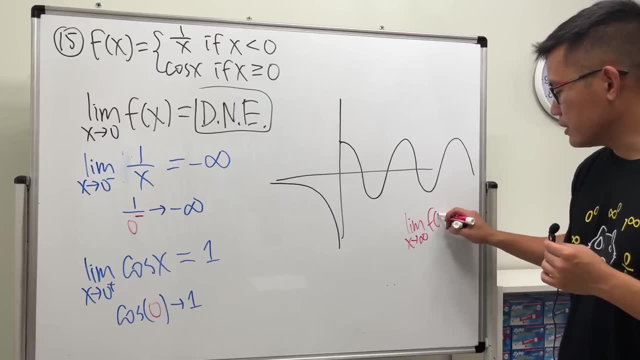 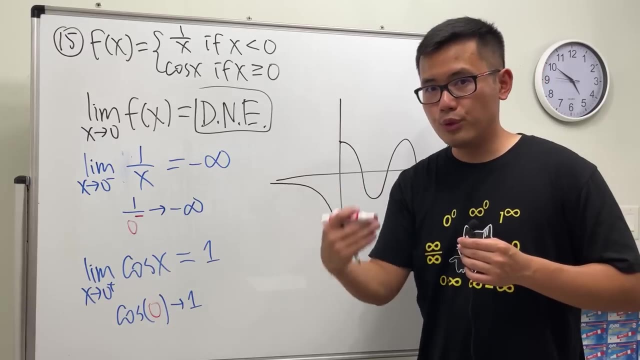 up and then like this: That's it. And of course, you can also like worry about if the limit is x, approaching infinity of the function. what's the answer for this? Ah, doesn't exist either, right, because it keeps going up and down, up and down in between. 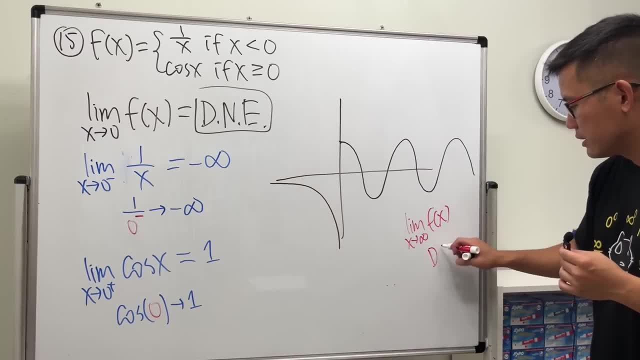 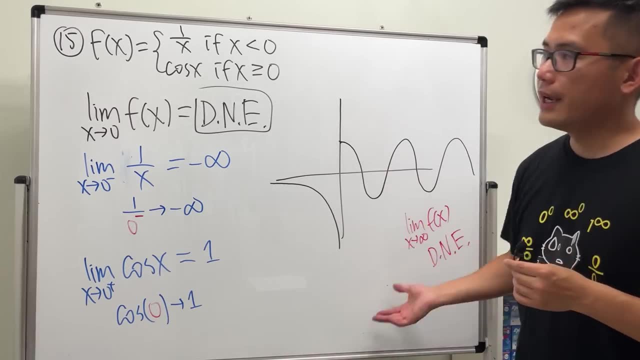 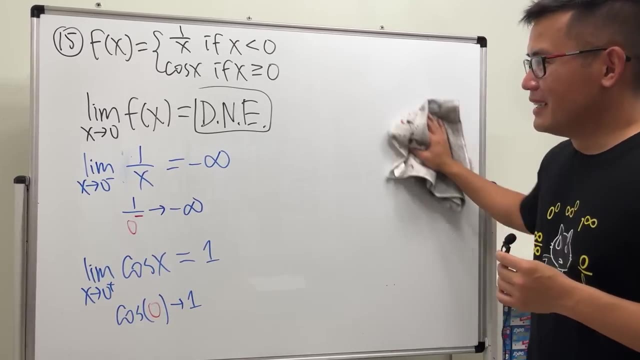 of negative Negative 1 and 1, the y value just bouncing right between negative 1 and 1, so no, Alright, number 15.. Okay, hopefully I don't need to like erase a question at every single time, because 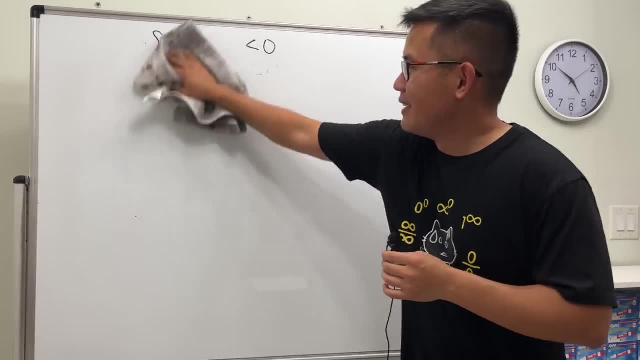 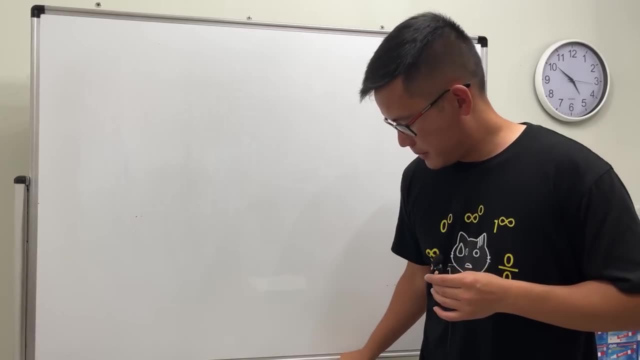 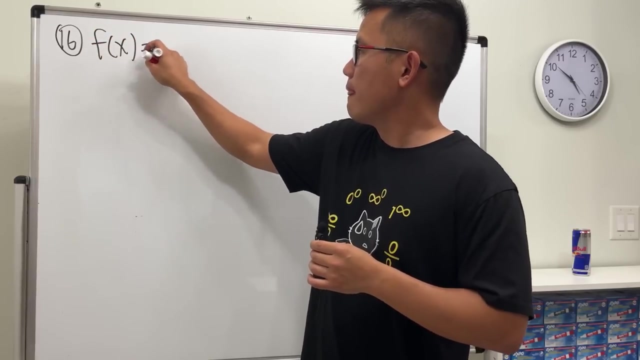 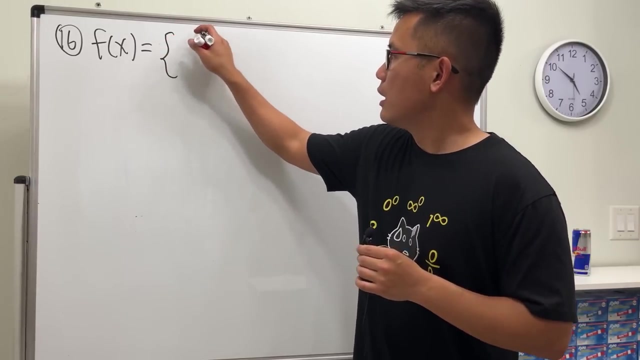 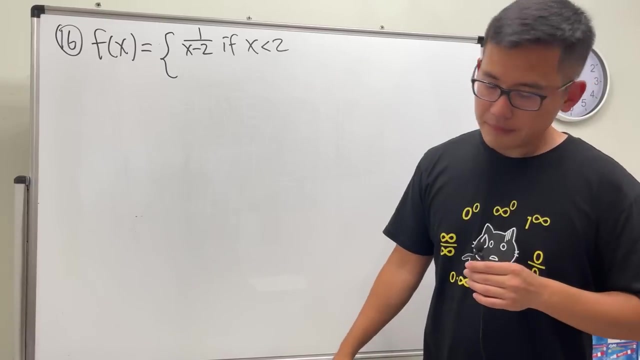 oh no, for number 16, I still have to make use of the whole board, but we will see Number 16,. our function is 1 over x minus 2.. This is when x is less than 2, and then ln of x minus 2, this is when x is greater than. 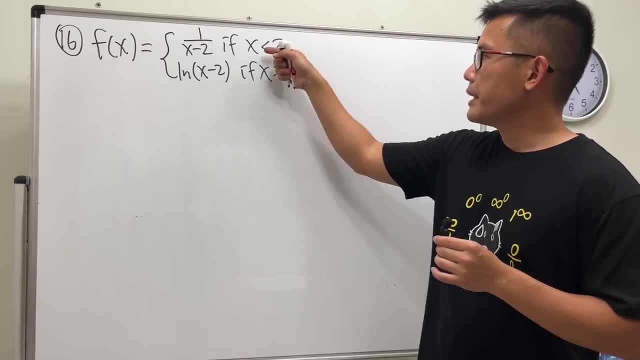 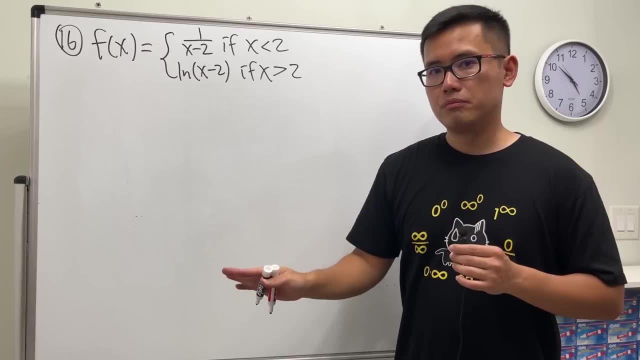 2. And notice: I cannot put equal sign For the first one. what for the second one? If I put equal sign right here, well, we cannot divide it by 0. And if I put equal sign here, that's also no good, because ln 0 isn't defined. 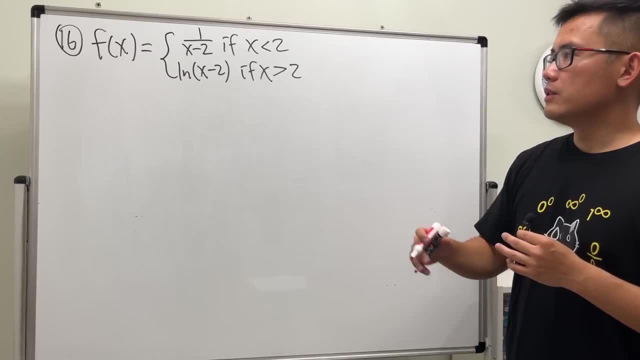 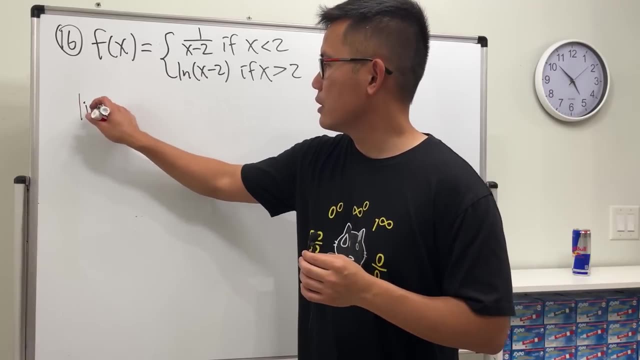 So here, f of x: right, the domain for x cannot be equal to 2.. But let's see, we want the limit as x approaching 2 of the function. And you know it. let's do exactly what we did. 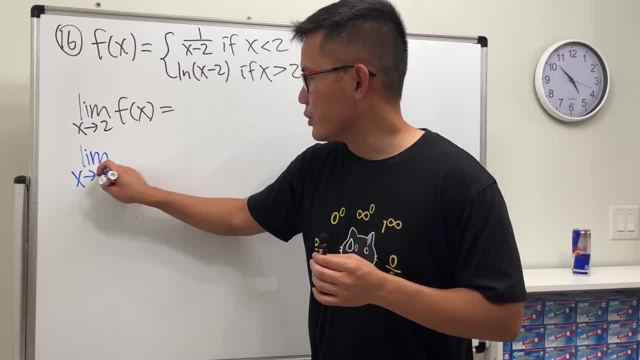 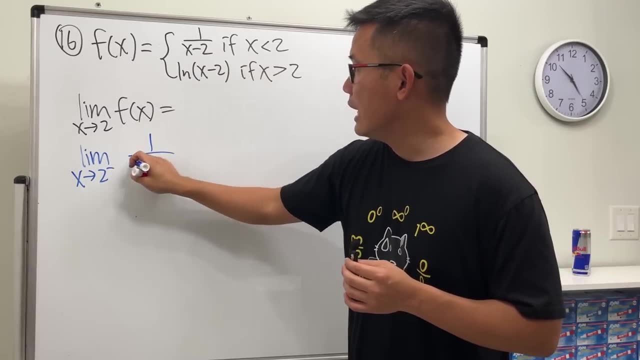 So here Take a look at the limit as x approaching 2 from the left-hand side first. If it's the left-hand side, then we are looking at this right here. So that's 1 over x minus 2.. 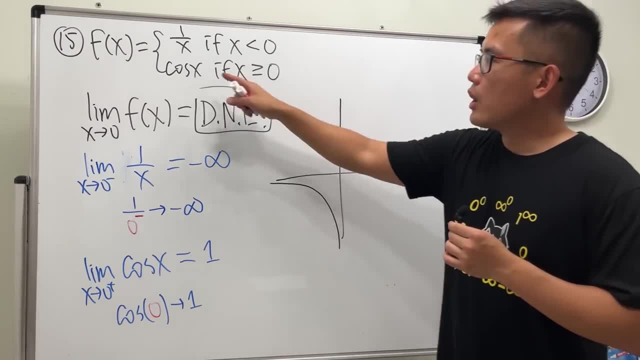 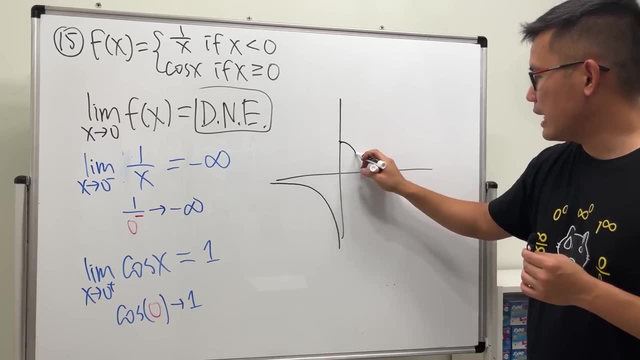 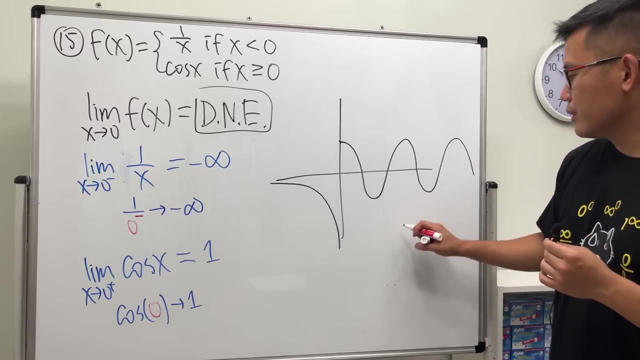 about when x is less than zero. so just this part. cosine x, cosine start with 0 comma 1, right, so we start right here and then it goes down up and then like this: that's it. and of course you can also like worry about if the limit is x approaching infinity of the function. what stands for this? 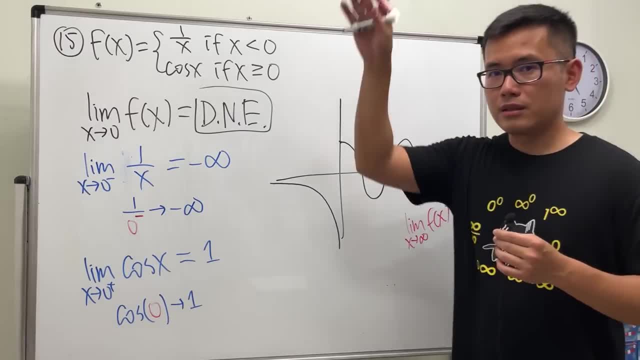 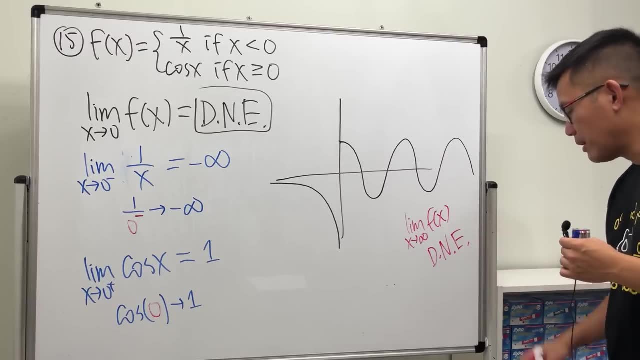 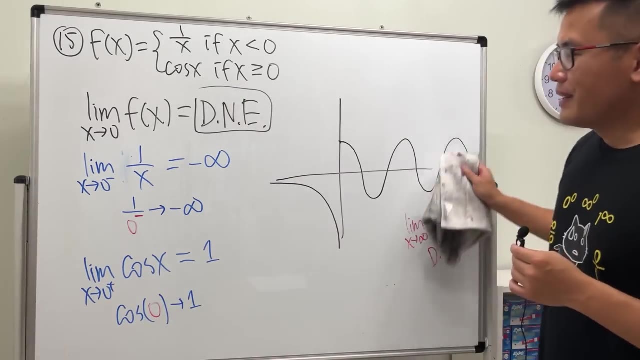 ah, doesn't exist either. right, because it keeps going up and down, up and down in between negative one and one, the y value just bouncing right between negative one and one. so, no, all right, number 15.. okay, hopefully i don't need to like erase a question at every single time, um. 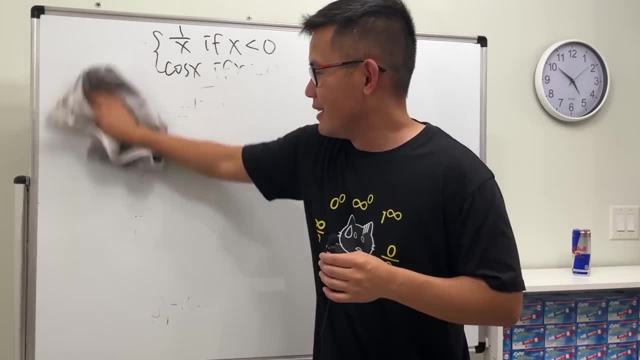 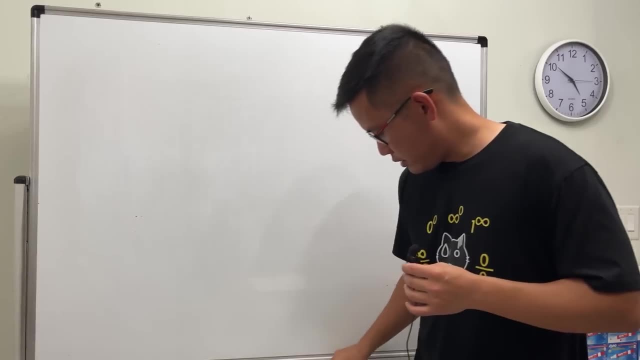 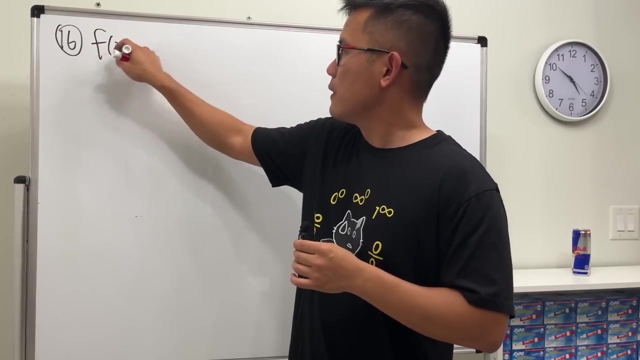 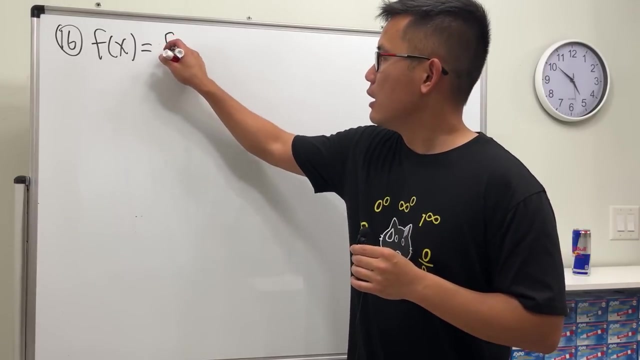 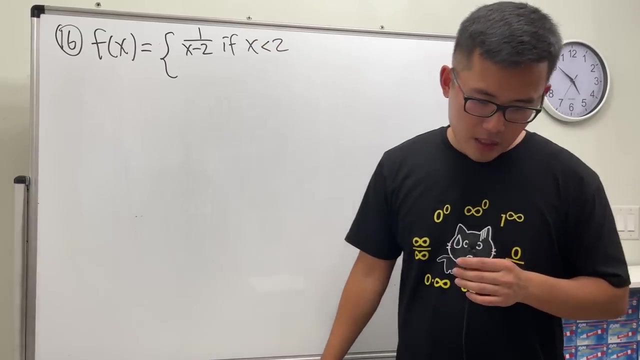 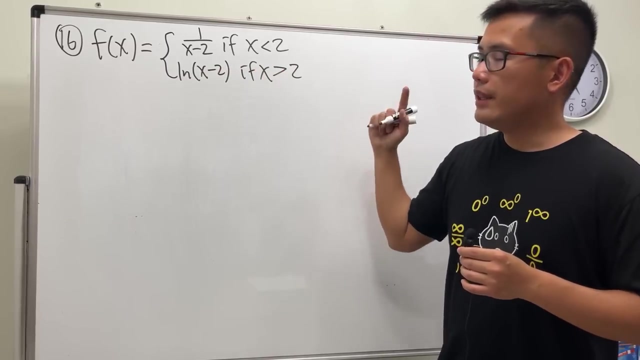 but because, oh no, for number 16 i still have to make use of the whole board. but uh, we will see number 16. our function is: 1 over x minus 2- this is when x is less than 2, and then ln of x minus 2. this is when x is greater than 2. and notice, i cannot put equal sign. 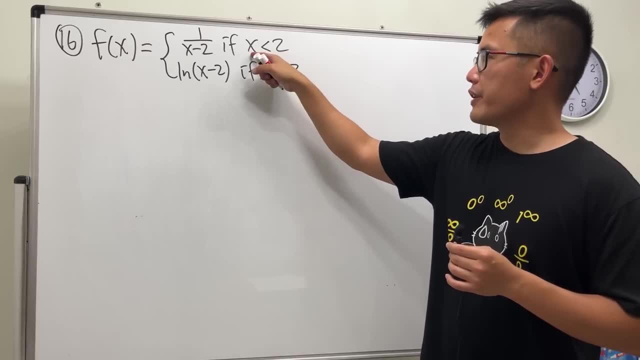 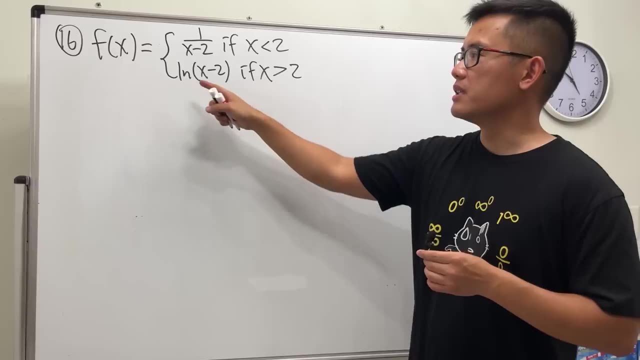 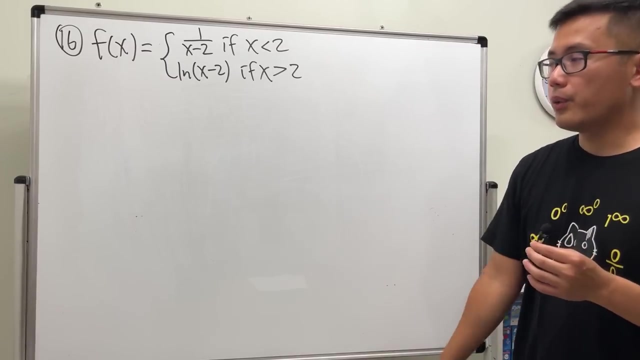 for the first one? what for the second one? if i put equal signs right here, well, we cannot divide it by 0. and if i put equal sign here, that's also no good, because ln. 0 isn't defined. so here f of x, right, the domain for it. x cannot be equal to 2.. 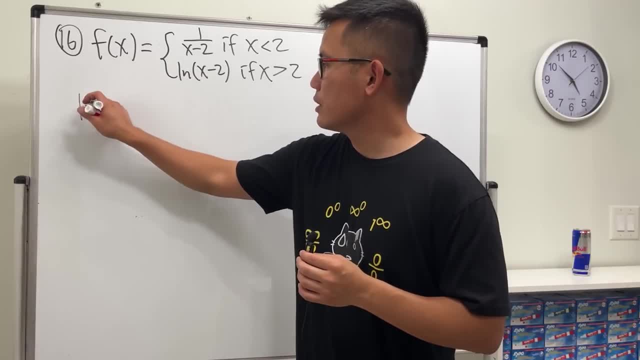 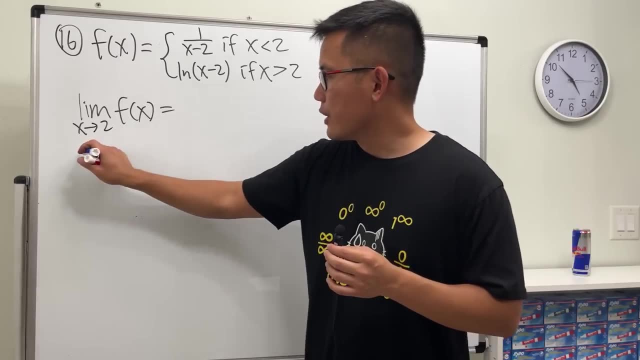 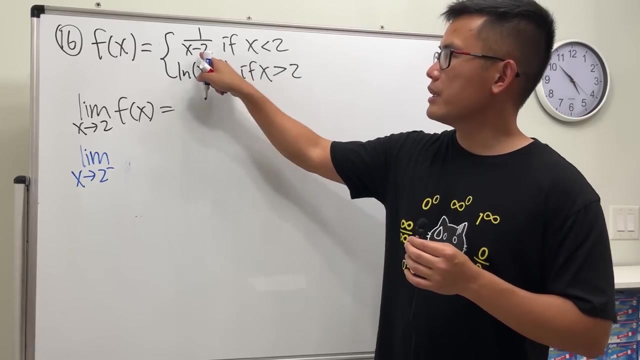 but let's see we want the limit as x approaching two of the function, and you know it. let's do exactly what we did so here, take a look at the limit as x approaching 2 from the left hand side first. if it's the left hand side, then we are looking at this right here. so that's. 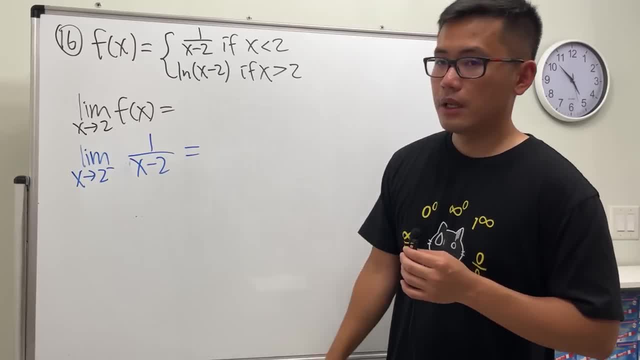 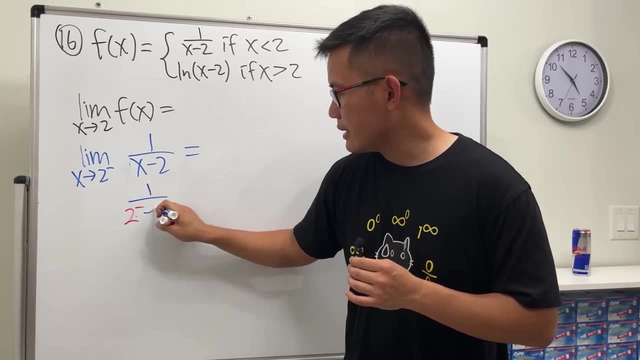 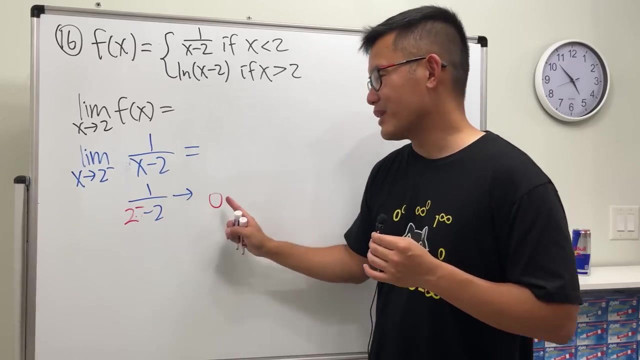 1 over x, minus 2.. okay, so put negative, put two minus in here, so we look at one over two minus, and then minus x is greater than 2 on this one, then favorite will go to the front right minus two. two minus two is zero, yes, but this is a little bit less than two. so this right here is: 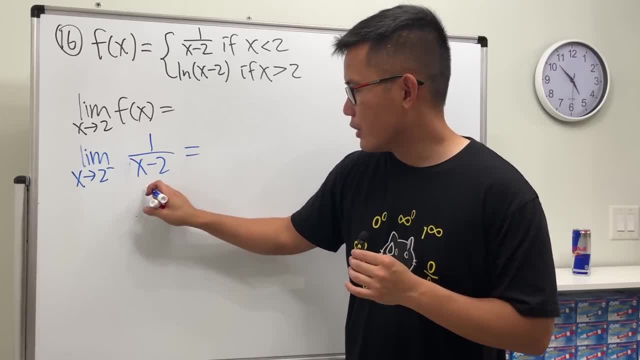 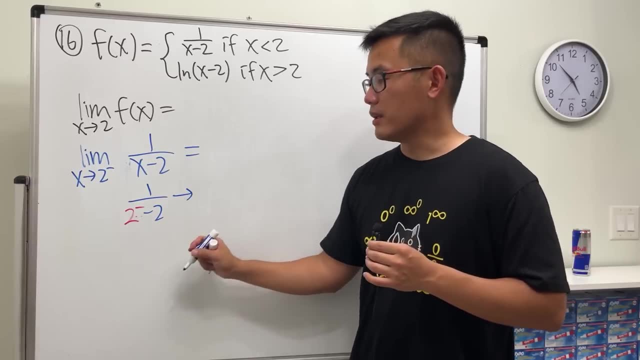 Okay, so put negative, put 2 minus in here. So we look at 1 over, 2 minus and then minus 2.. 2 minus 2 is 0, yes, But this is a little bit less than 2.. 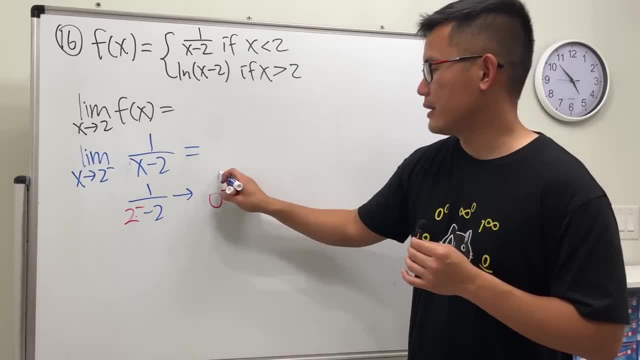 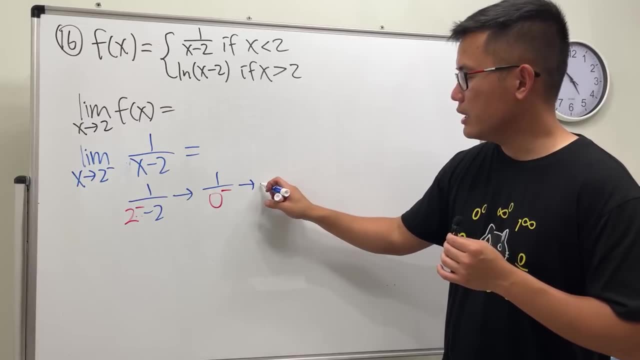 So this right here is technically 0 minus. Alright. so 1 over, 0 minus. This is positive, this is negative And the limit 4 on the bottom is 0, right, So altogether we get negative infinity. 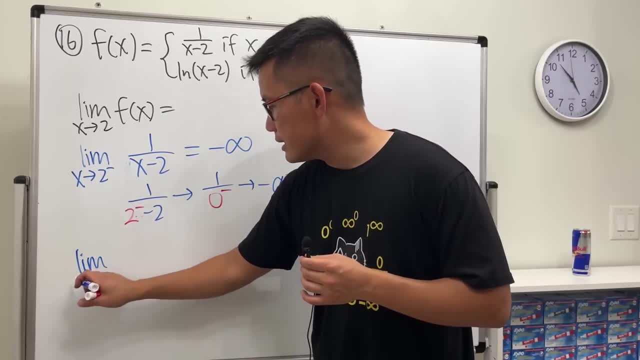 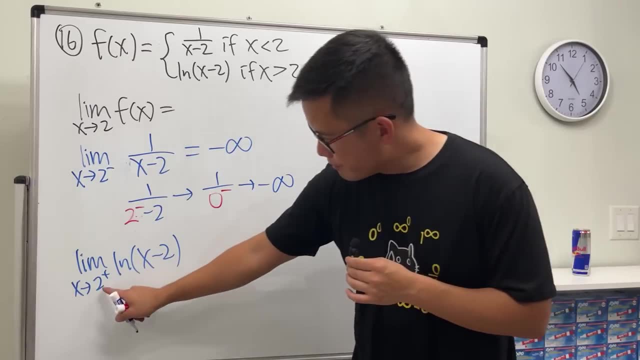 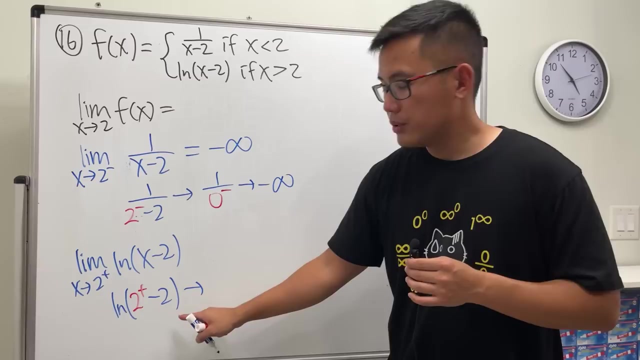 Okay. Secondly, limit as x approaching 2 plus, then we are looking at ln of x minus 2.. Well, put 2 plus in here we get ln of 2 plus minus 2.. 2 minus 2 is 0, but this is a little bit bigger than 2.. 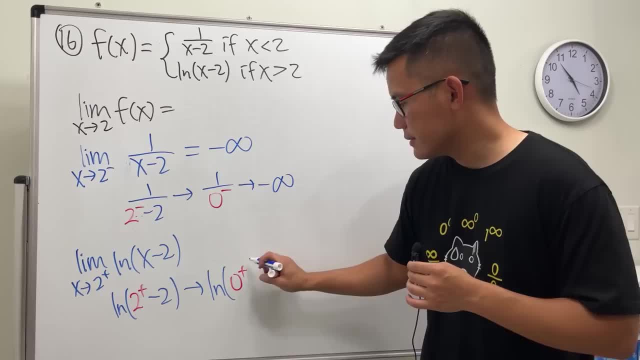 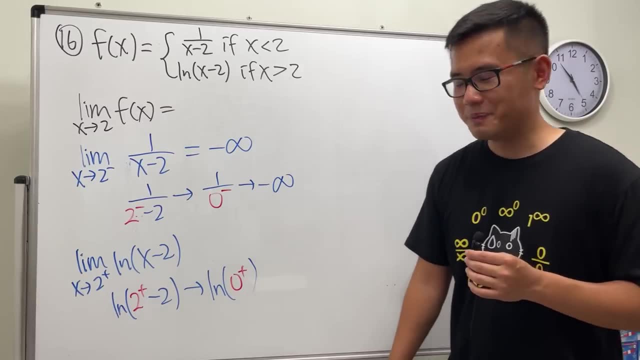 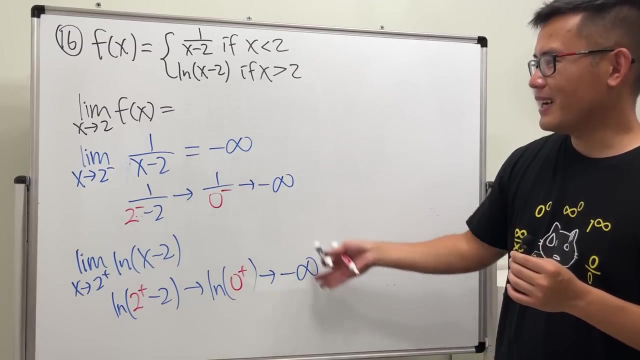 So the inside is: It's technically 0 plus What's ln of 0 plus? Remember the things that we talked about maybe like 14 minutes ago? This right here approaches negative infinity. So, surprise, They are the same. 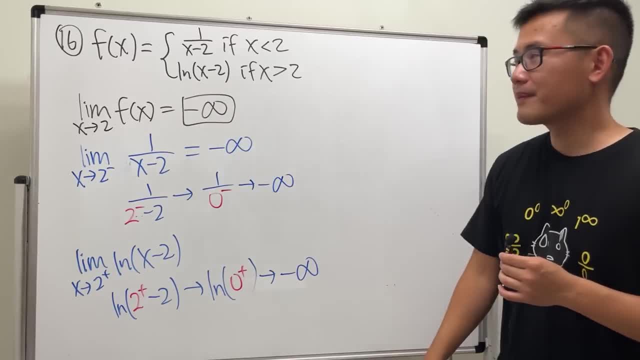 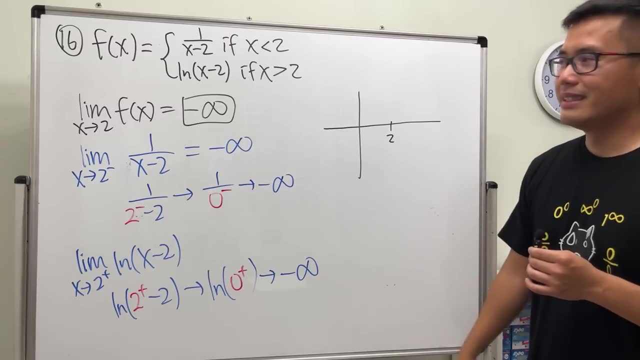 So the answer is actually negative infinity. Okay, Alright, so just real quick. How does the graph of this look when x is 2? 1 over, Remember x minus 2?? It has a vertical isotope, and then the picture looks like this: 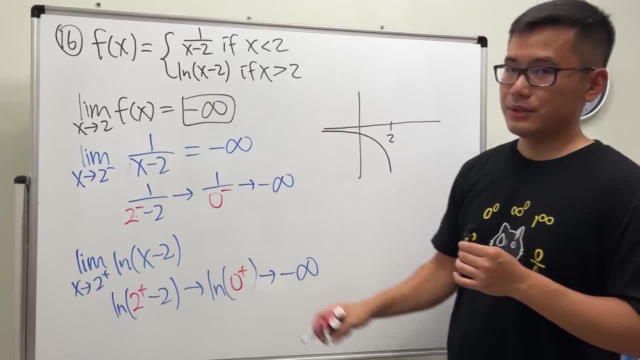 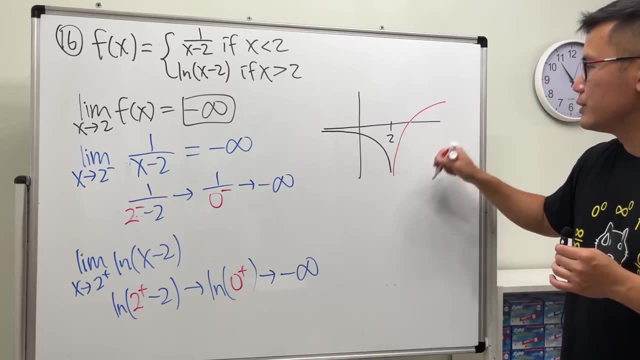 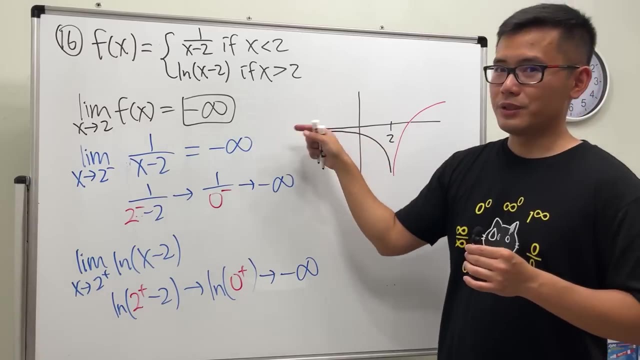 Okay, ln of x minus 2.. ln of x minus 2.. Also vertical isotope, And It's actually like this, Because, remember, ln of x, it actually grows to infinity right, So it actually goes up. But this piece, it has a horizontal isotope. 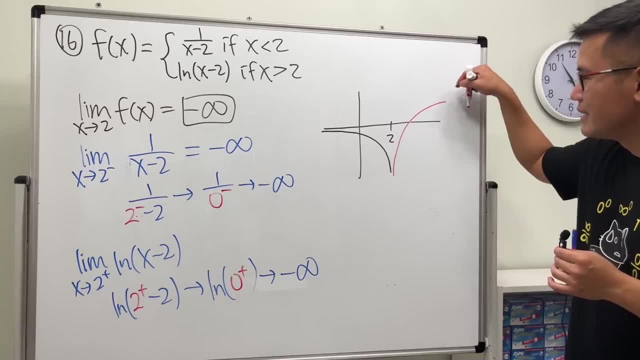 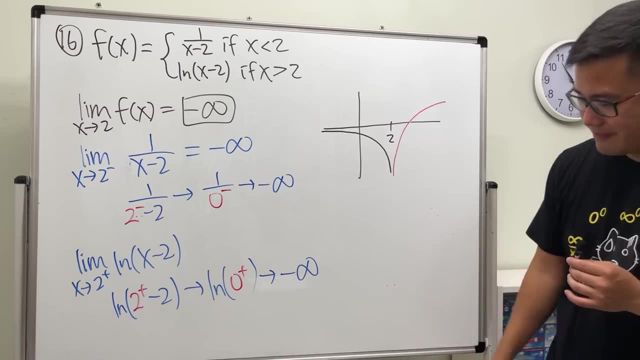 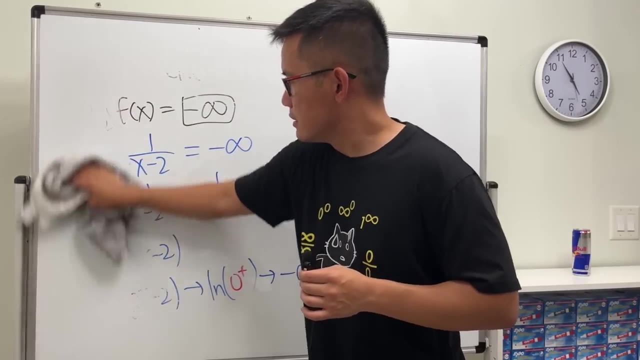 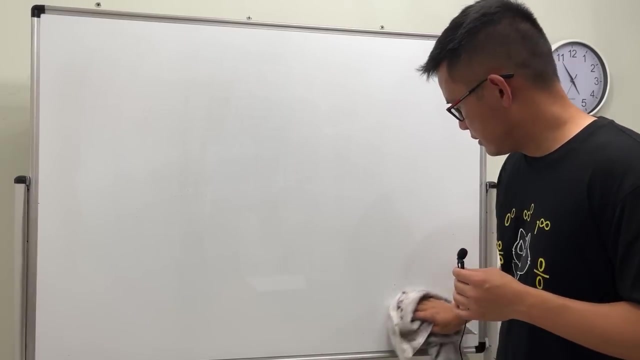 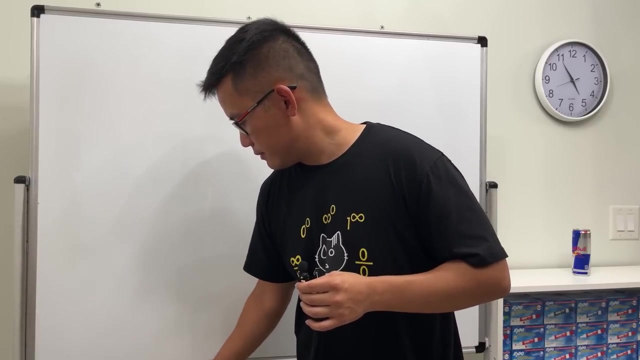 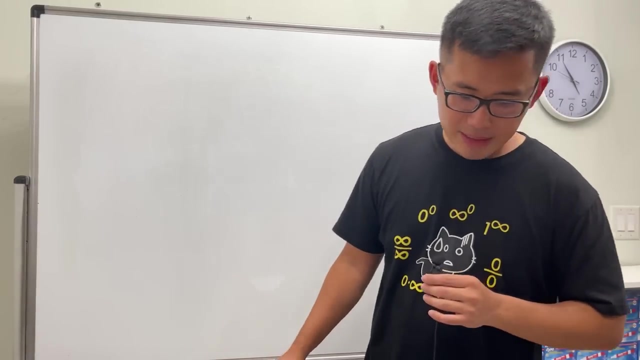 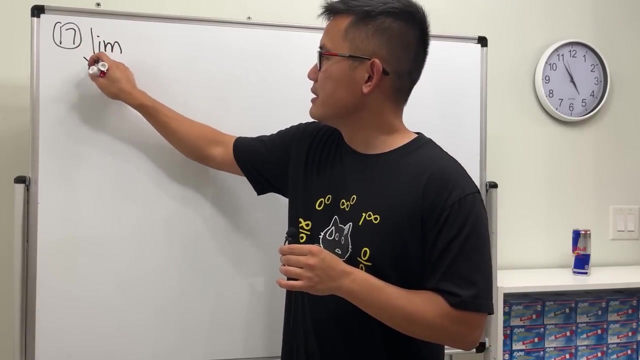 This one does not, So it's a pretty cool curve. This is the ln x minus 2.. And this is the rational function: 1 over x minus 2.. Stop the function. Okay, Thank you all. right, number 17. here's the deal. we are just going to evaluate the limit as. 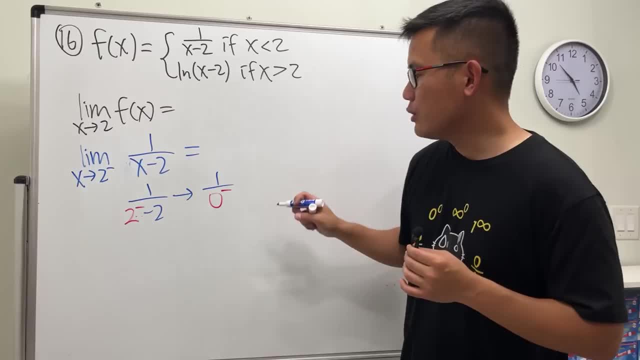 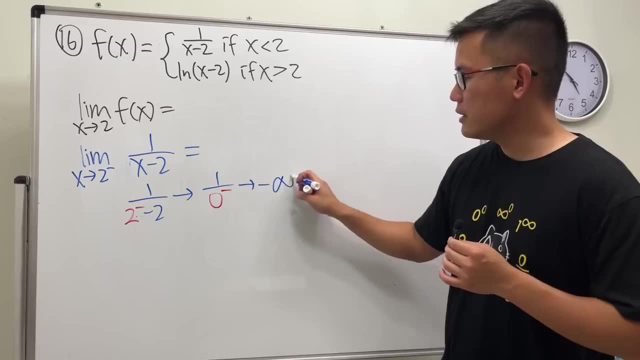 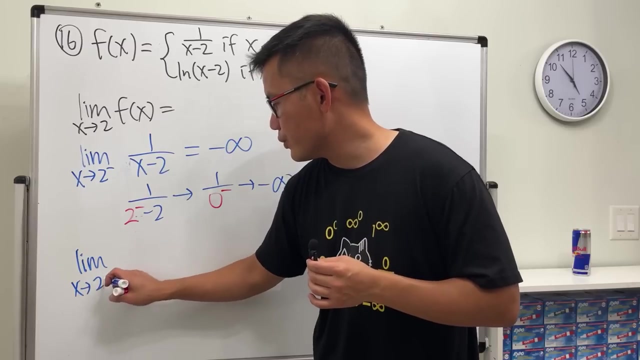 technically zero minus, all right. so one over zero minus. this is positive, this is negative, and the limit four on the bottom is zero, right, so altogether we get negative infinity, okay. secondly, limit as x approaching two plus. then we are looking at ln of x minus two. 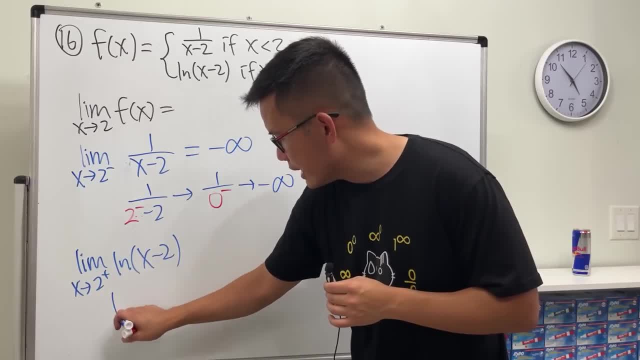 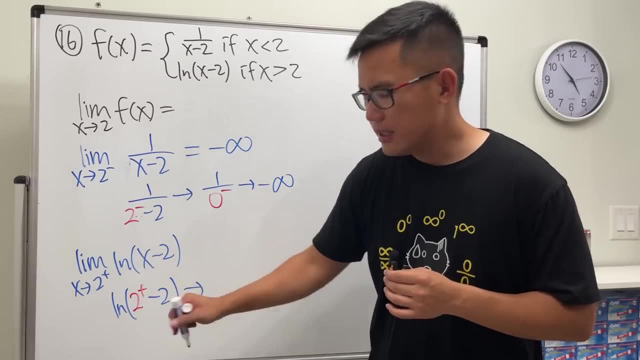 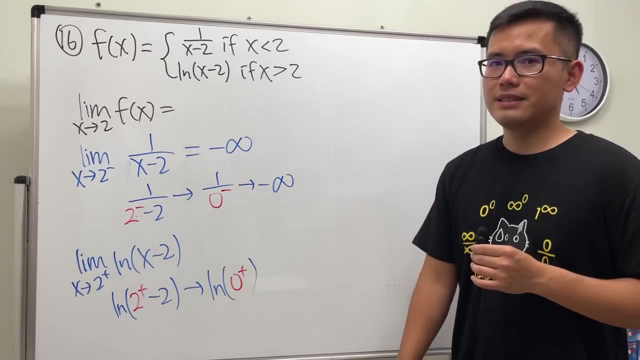 well, put two plus in here we get ln of two plus minus two. two minus two is zero, but this is a little bit bigger than two, so the inside is technically zero plus. what's ln of zero plus? remember the things that we talked about maybe like 14 minutes ago? this right here approaches. 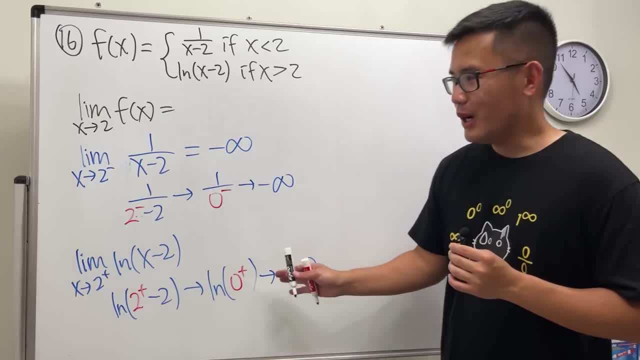 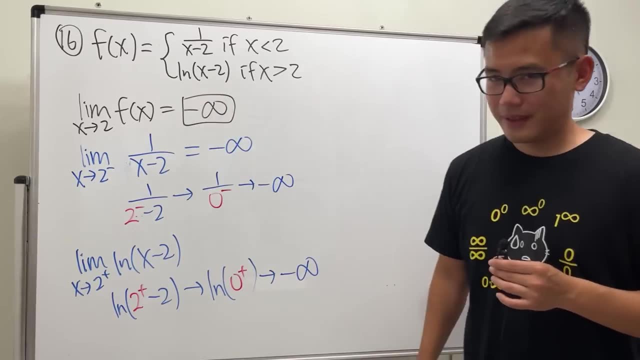 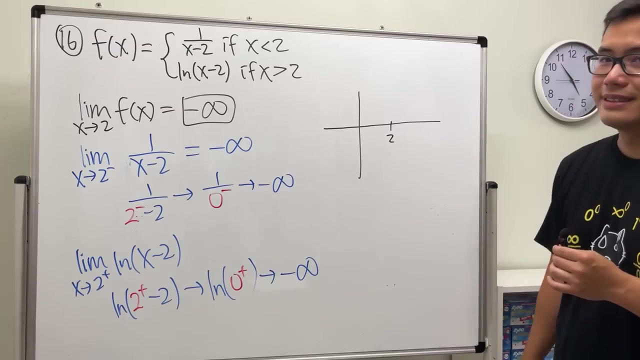 negative infinity. so, surprise you, they are the same. so the answer is actually negative infinity. okay, all right. so just real quick, how does the graph of this look when x is two, one over x minus two? it has a vertical isotope, and then the picture looks like this: 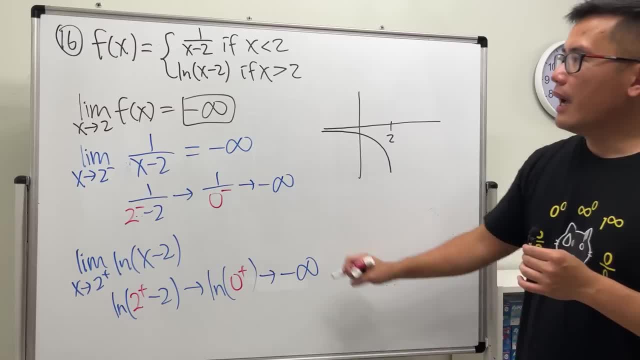 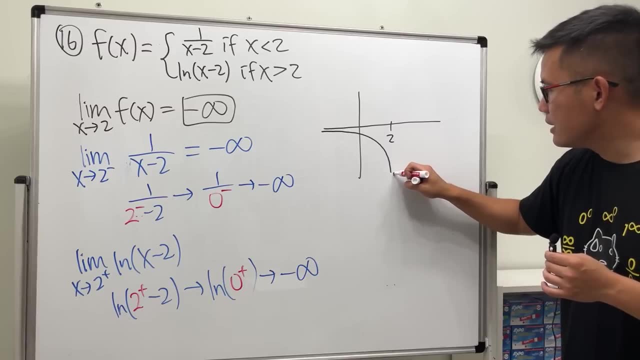 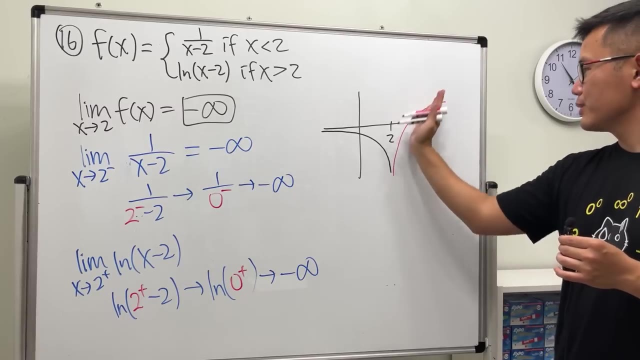 okay, ln of x minus two, ln of x minus two, also vertical isotope. and then the picture looks like this: because remember ln of x, it actually goes to. because remember ln of x, it actually grows to infinity. right, so it actually goes up. but this piece it has a horizontal 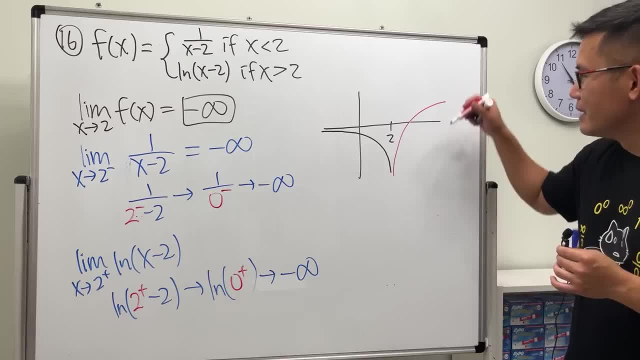 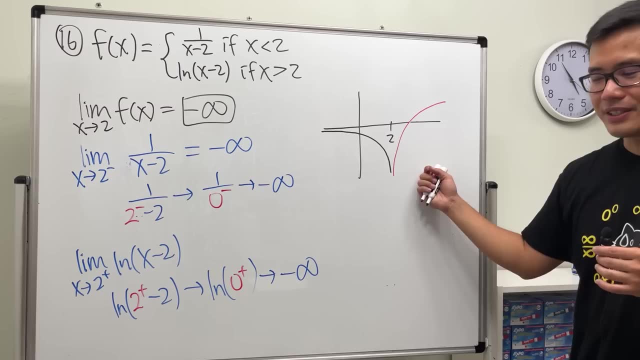 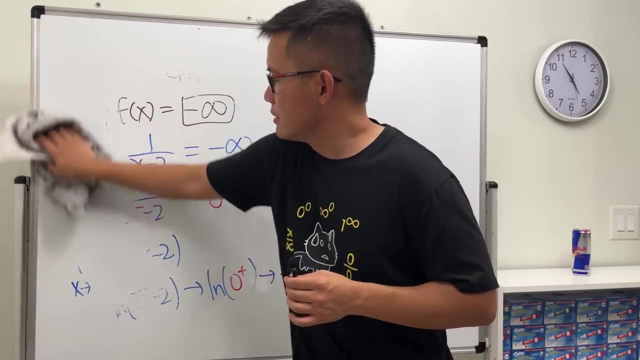 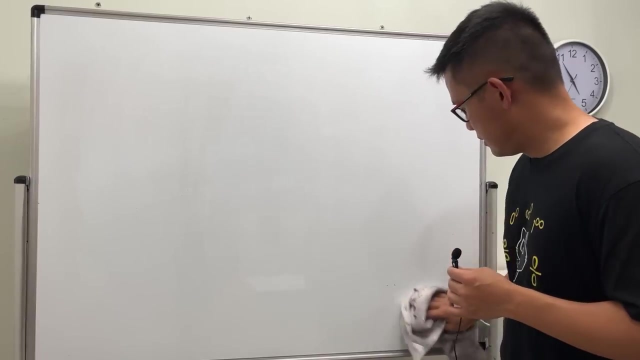 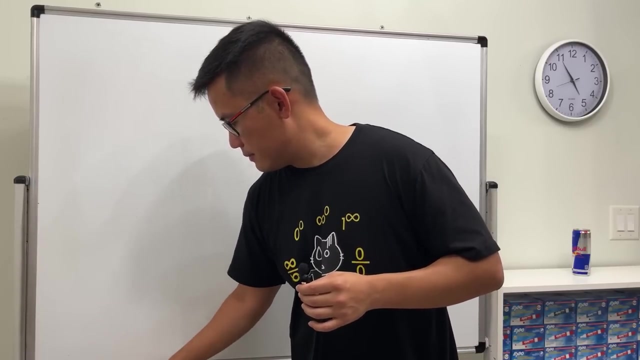 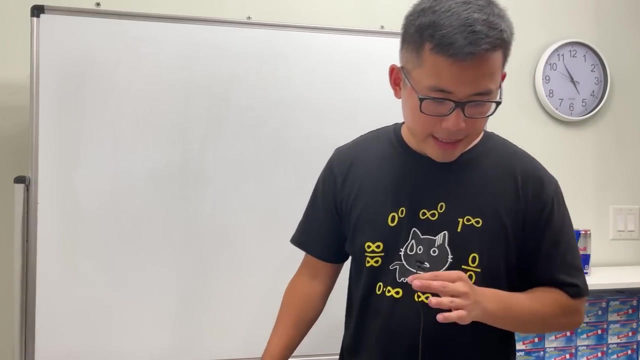 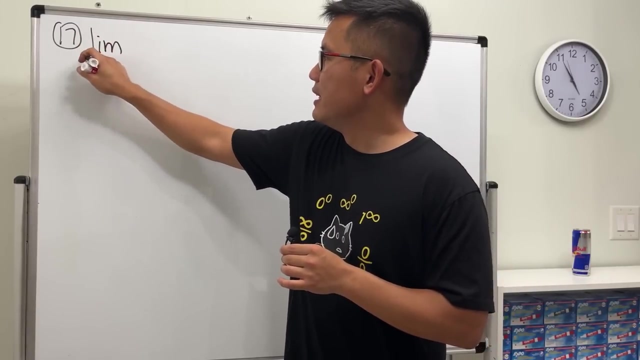 staple. this one does now. so it's a pretty cool curve. this is the ln x minus two part and this is the rational function one over x minus two. just stop the function. stop the function. all right, number 17: here's the deal. we are just going to evaluate the limit as x. 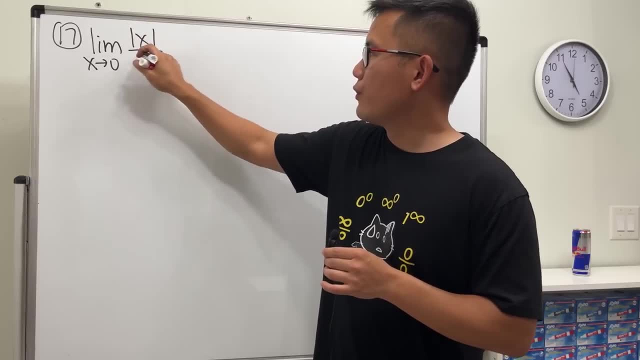 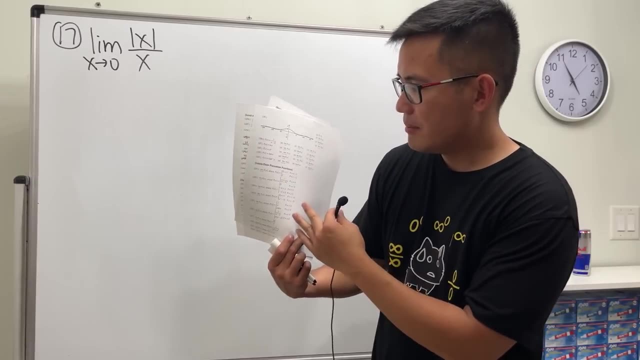 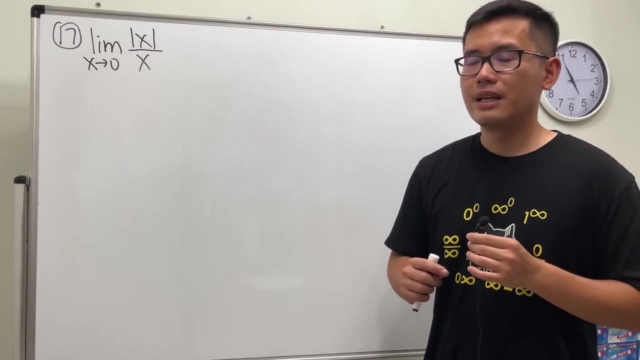 approaching 0 and i give you absolute value of x over x. did i make a mistake? this category? i'm saying that it's the limits from piecewise functions. i don't see no piecewise functions. technically. there is because when we have absolute value of x, it's technically an absolute. 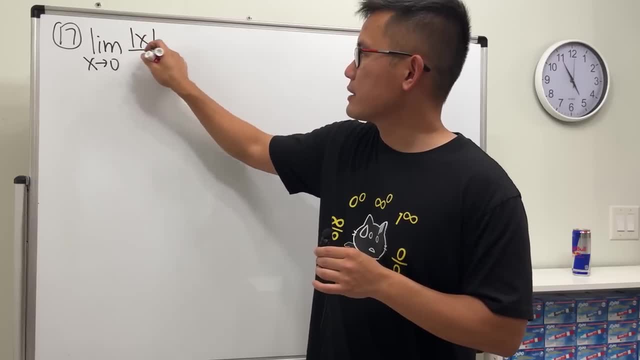 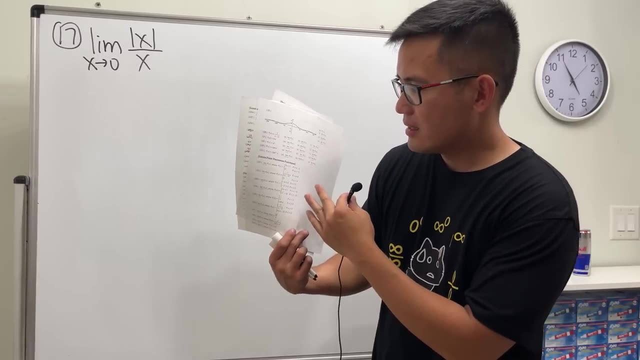 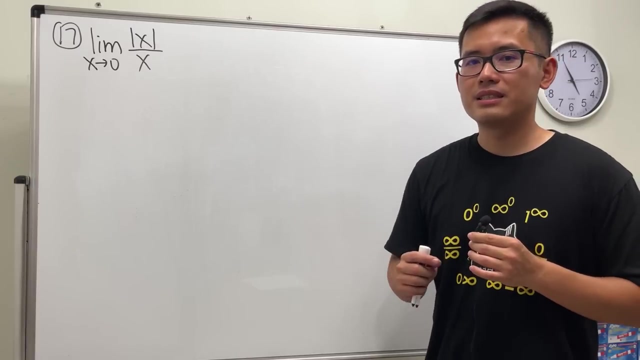 X approaching 0 and I give you absolute value of X over X. Did I make a mistake? this category? I'm saying that it's the limits from piecewise functions. I don't see no piecewise functions. technically there is because when we have absolute, 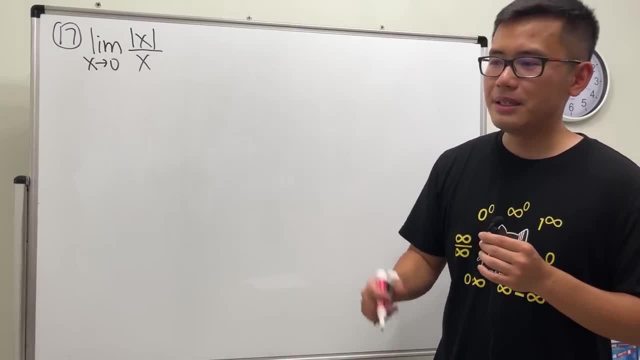 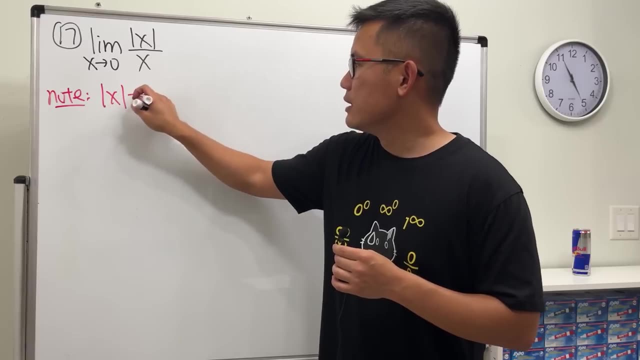 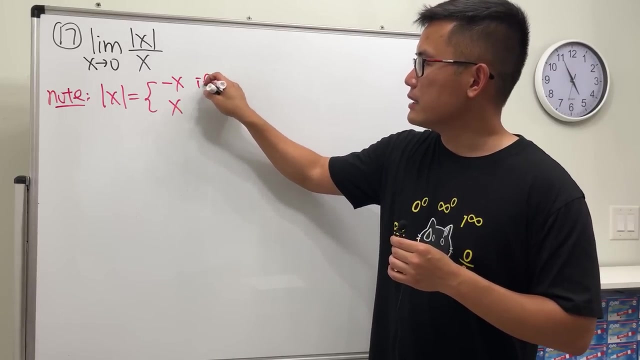 value of X. it's technically an absolute value. it's technically a piecewise function. so I would like to write this down right here for you guys. note, when we have absolute value of X, this actually means either we get negative X or positive X. we get negative X when the inside named X is negative because 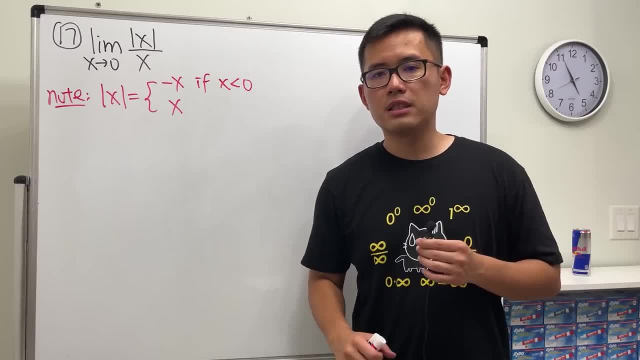 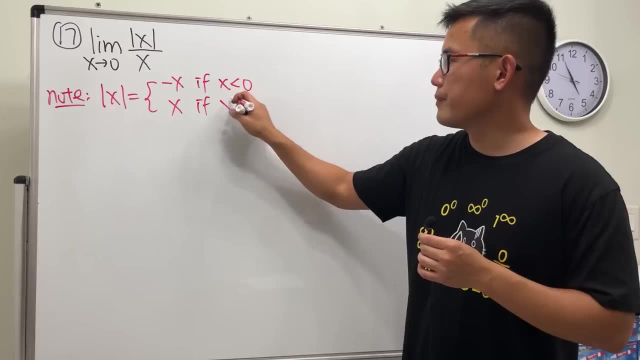 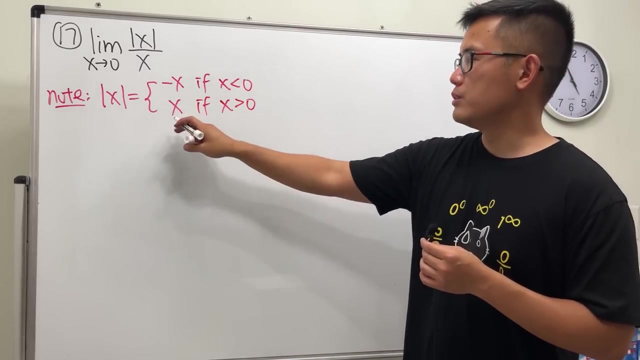 negative times negative. that's how we can produce a positive output. and if the inside is already positive, then we just, you know, have the X back. and the truth is, you can put a equal sign here or here, doesn't matter, because 0 is still negative, 0 is still 0, but usually 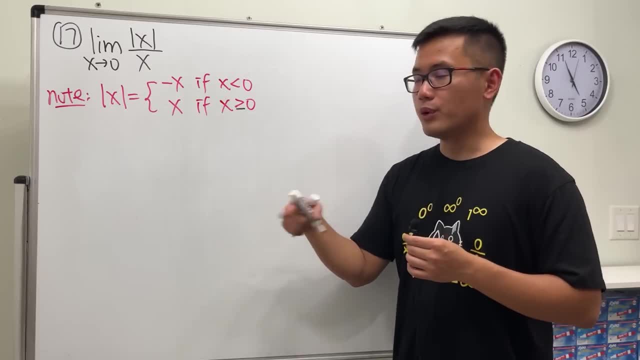 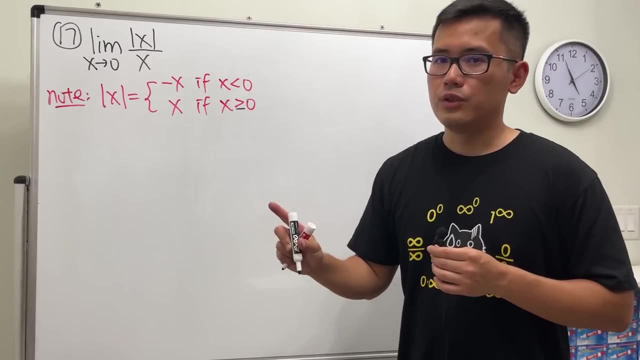 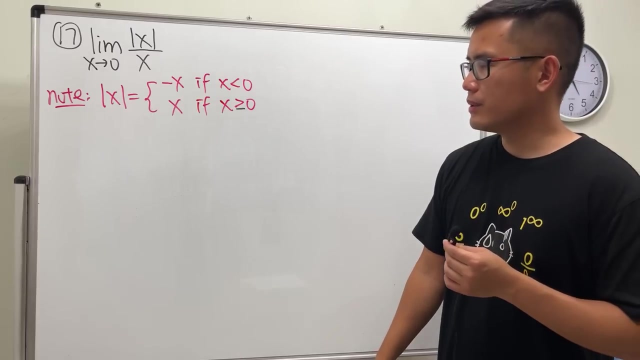 people put equal sign there. all right, so let's see this right. here is our piecewise definition, but we want absolute value of X over X, so how exactly do we do this? we have to check this out. when we have absolute value of X over X? this right. 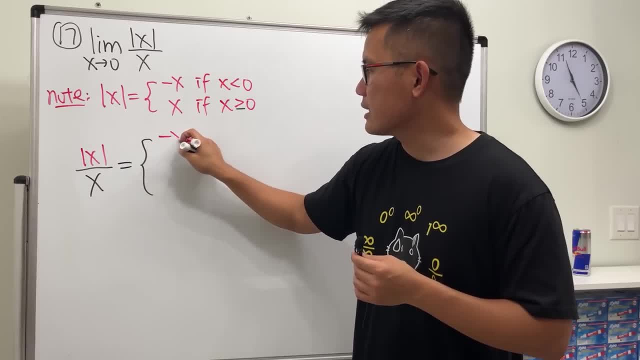 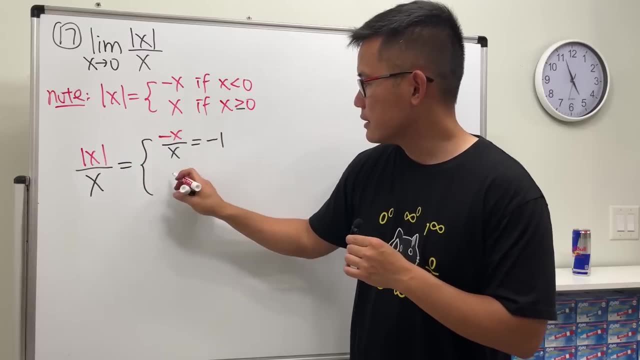 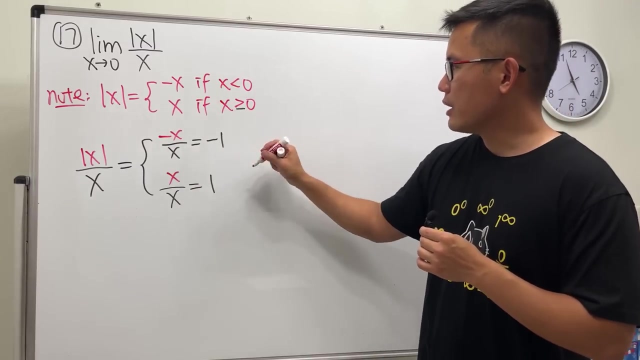 here we can just go ahead and do negative X divided by this X, and this is going to reduce to negative 1. similarly, we do X divided by this X, and this right here will give us positive 1, but be careful though. this right here, yes, is. 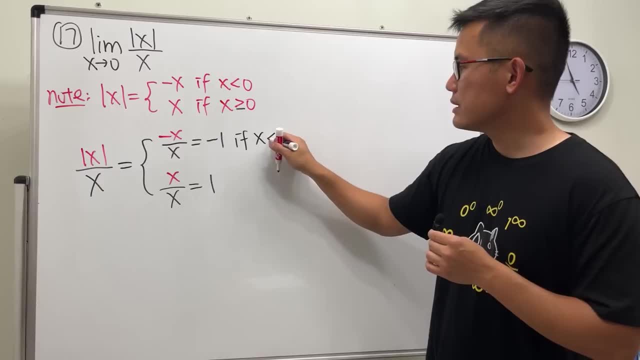 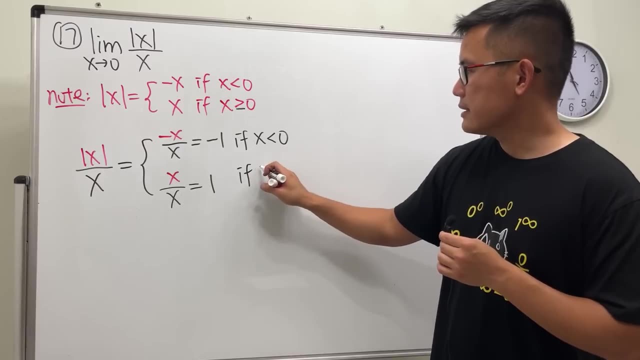 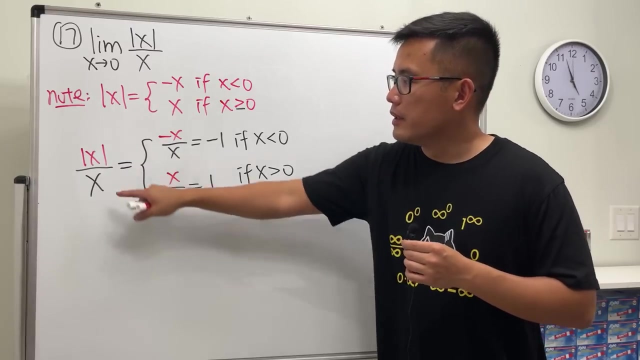 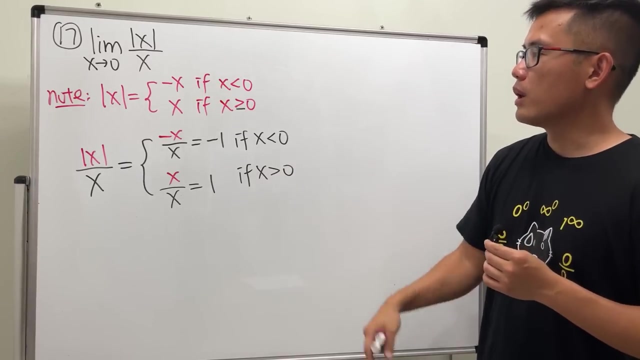 still if X is less than zero. however, for this right here, this is: if X is greater than 0. no more equal sign. we cannot use equal sign anymore because the expression right here has the X on the bottom. we cannot have 0 on the bottom, so we lose that equality. all right. 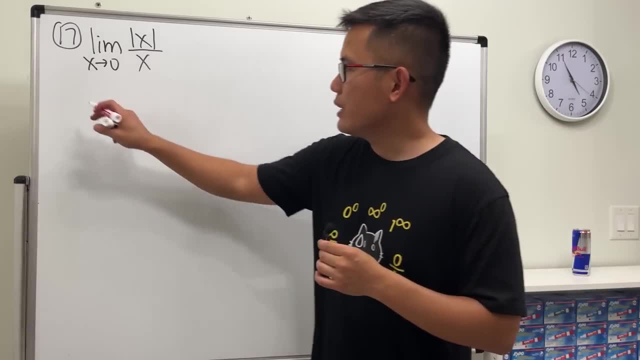 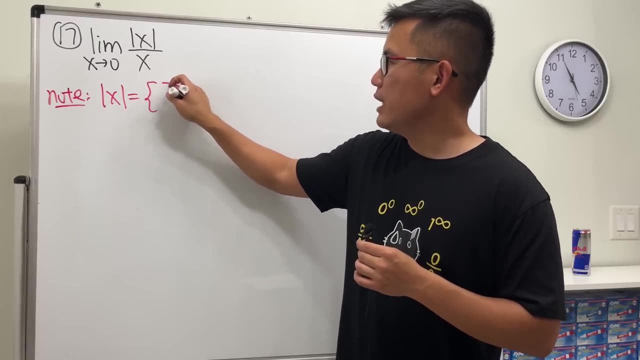 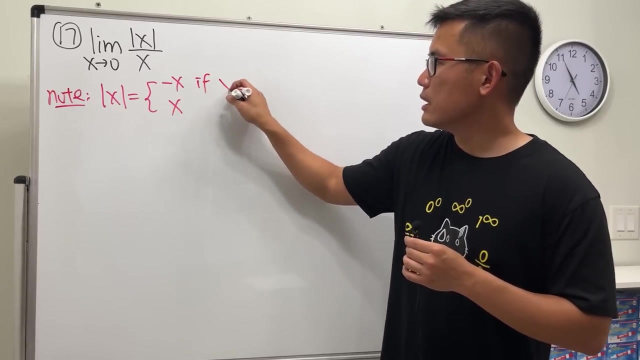 for your. it's technically a piecewise function, so i would like to write this down right here for you guys. note, when we have absolute value of x, this actually means either we get negative x or positive x. we get negative x. when the inside named the x is negative because negative times negative. that's how we can produce a positive. 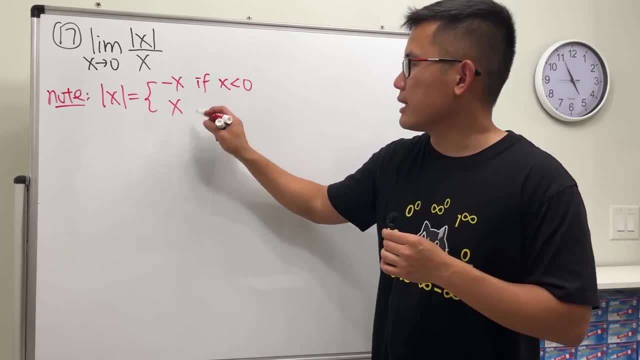 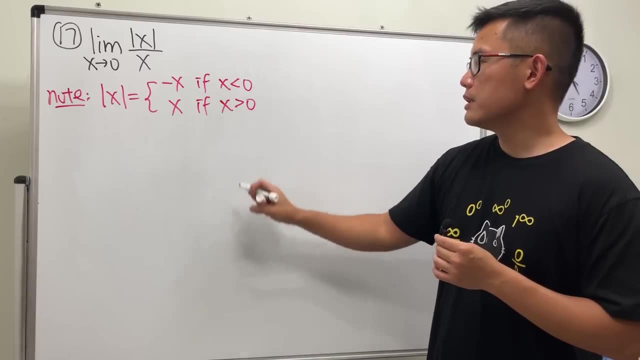 output, and if the inside is already positive, then we just, you know, have the x back. and the truth is, you can put a equal sign here or here, doesn't matter, because zero is zero. and you can put a equal sign here or here, doesn't matter, because zero is zero. 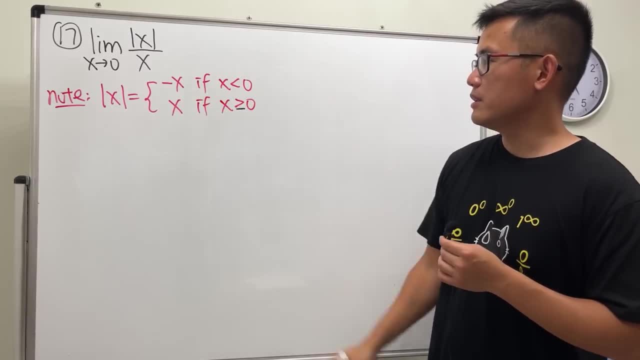 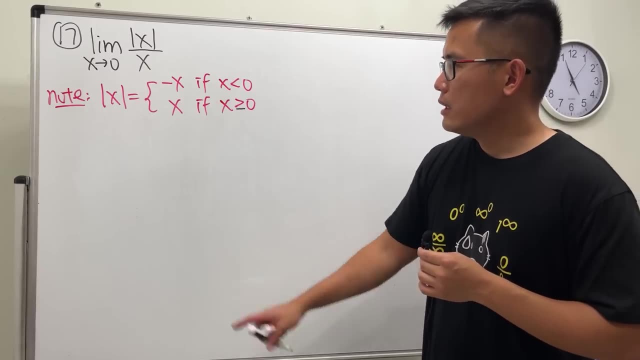 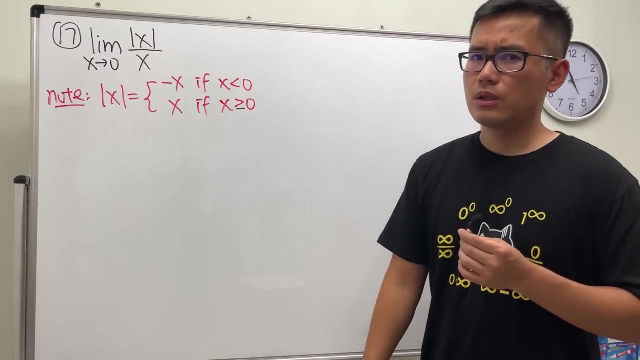 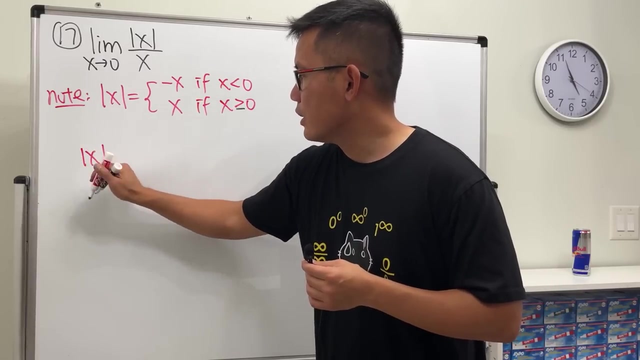 negative. zero, zero, she wrote, but usually people put equal sign there. all right, so let's see this right here at our p-square definition. but we want absolute value of X over X. so how exactly do we do this? well, check this out. when we have absolute value of X over X, this right here, we can just go ahead and do negative. 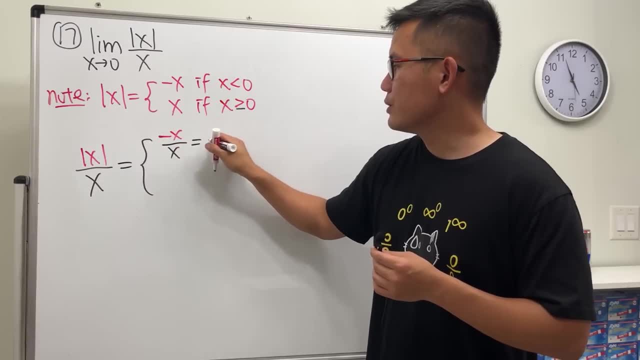 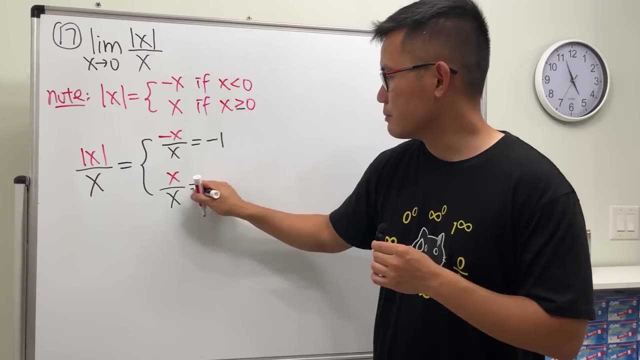 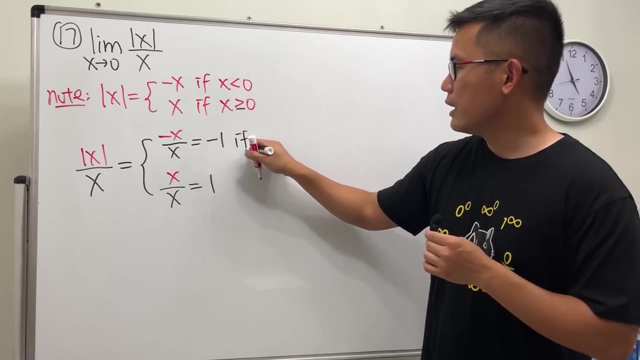 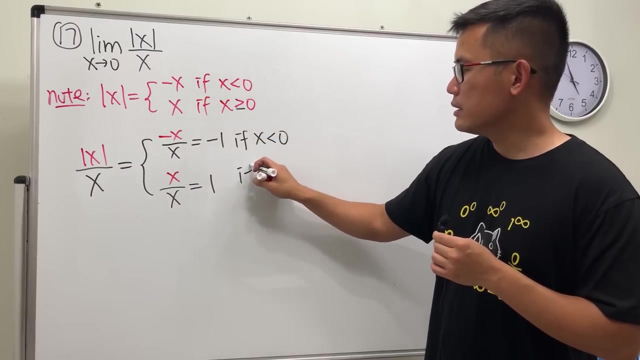 x divided by this x, and this is going to reduce to negative 1. similarly, we do x divided by this x, and this right here will give us positive 1, but be careful though. this right here, yes, it's still- if x is less than 0. however, for this right here, this is if x is greater than 0. 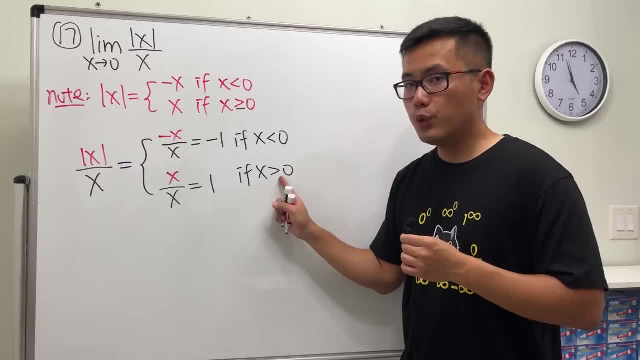 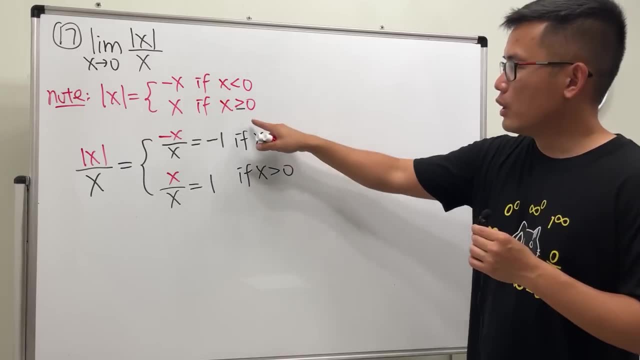 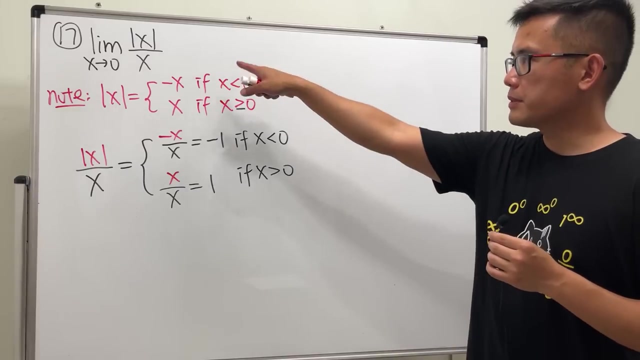 no more equal sign. we cannot use equal sign anymore because the expression right here has the x on the bottom. we cannot have 0 on the bottom, so we lose that equality. all right, so this is how you write up: p twice function for epsilon phi of x over x, and this right here. 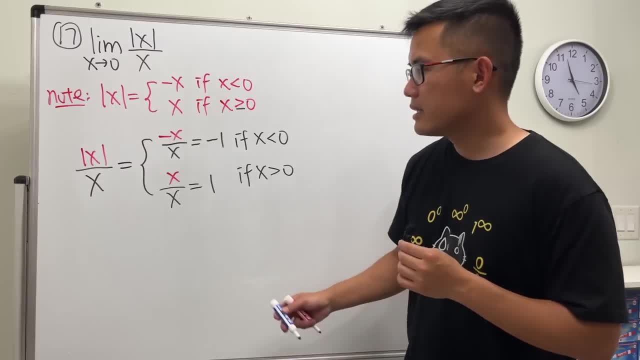 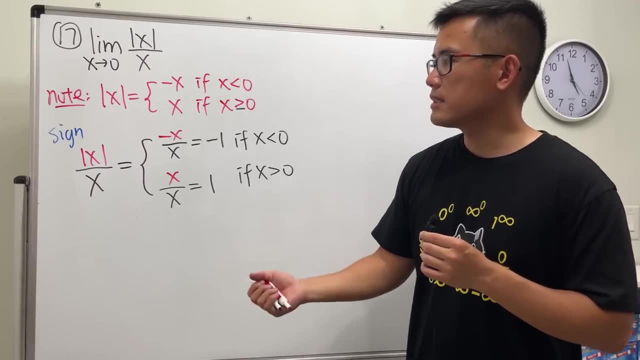 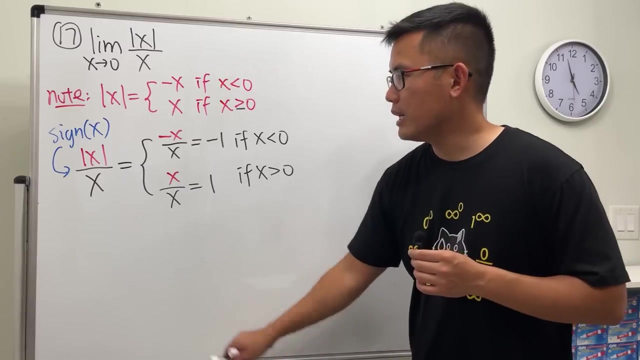 actually has a special name sign but, like the way you spell, it is s, i n g, because it tells you if it's like a positive sign. so if x is greater than 0, this is going to reduce to negative 1 positive or negative sign of the number x. so yeah, but anyway, though you don't have to know. 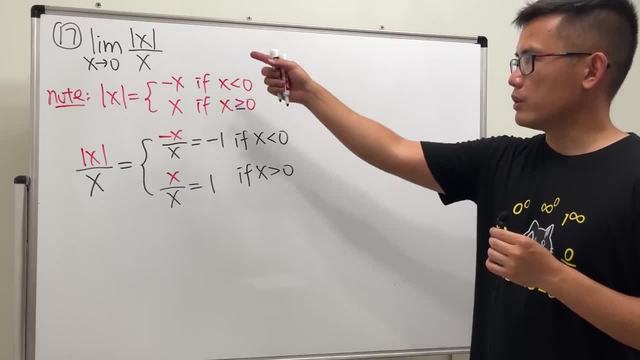 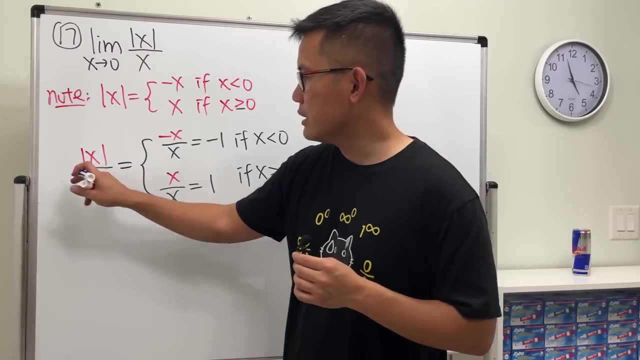 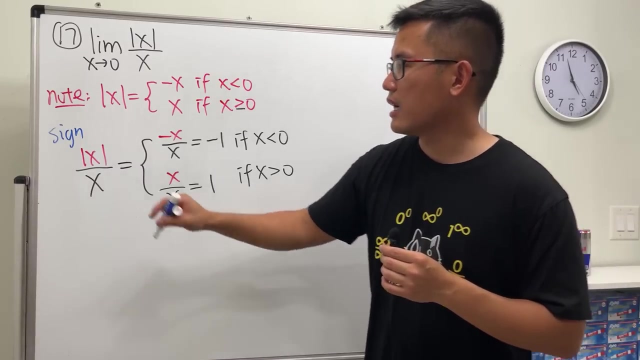 so this is how you write that piecewise function for F of X over X, and this right here actually has a special name, Stein, but like the way you spell, it is S I N G, because it tells you if it's like a positive or negative sign of the. 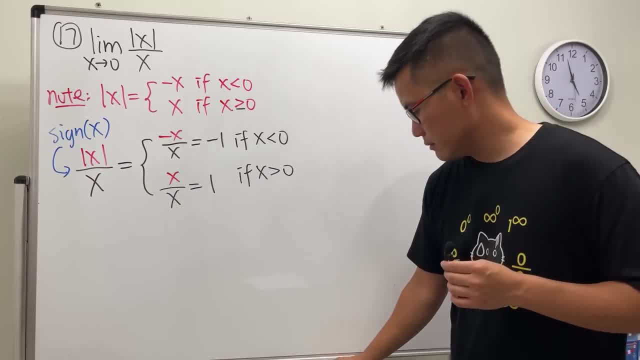 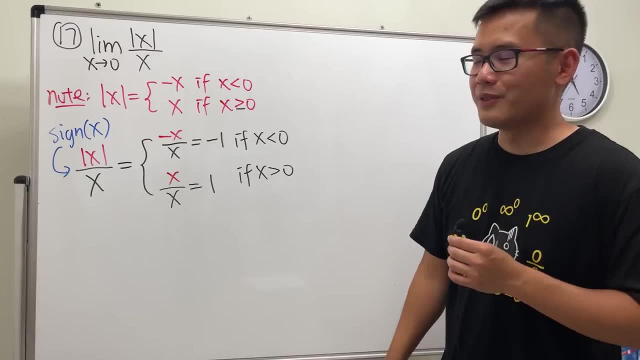 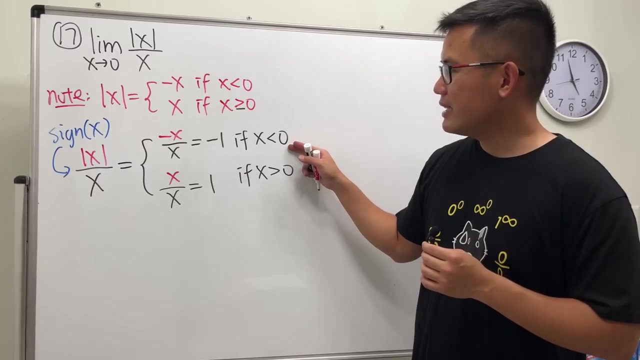 number X. so yeah, by anyway, though you don't have to know what I don't know depends on the teacher- but yeah, but you need to know this and the piecewise function for that. anyway, what's the answer for that? from the know Negative side, we get negative one. 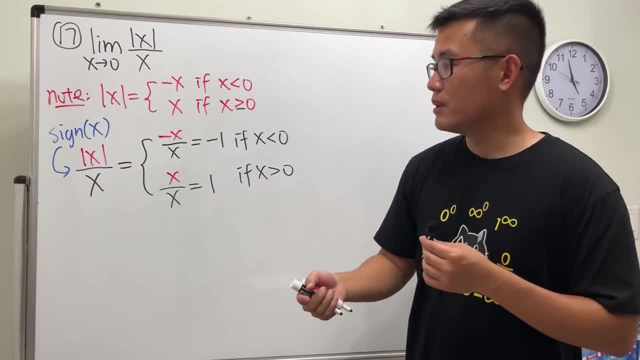 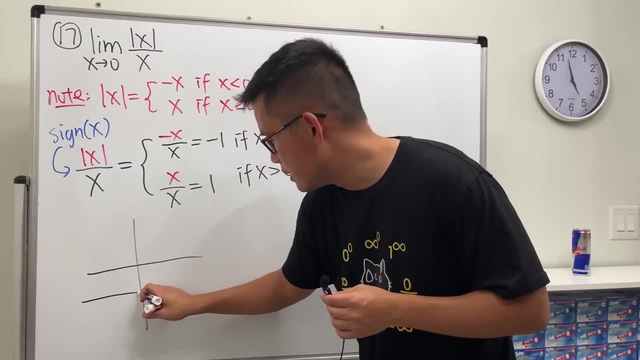 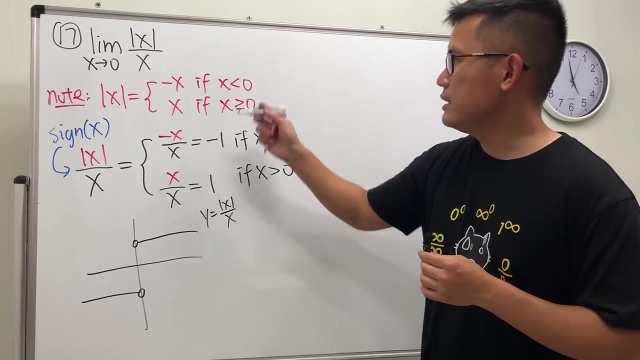 On the right-hand side, we get positive one, So they do not equal. You can make a graph of this real quick: Negative one and then one, And this is the graph for absolute value of x over x. But either way, though, this right here does not exist. 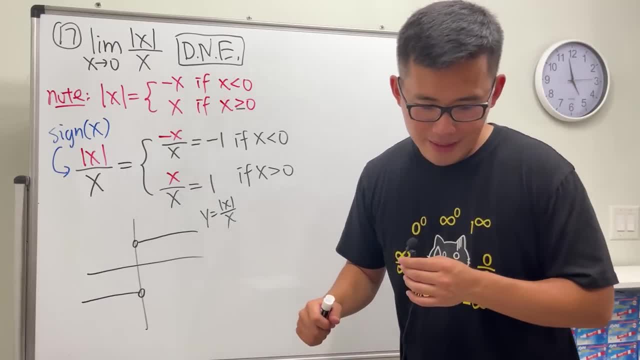 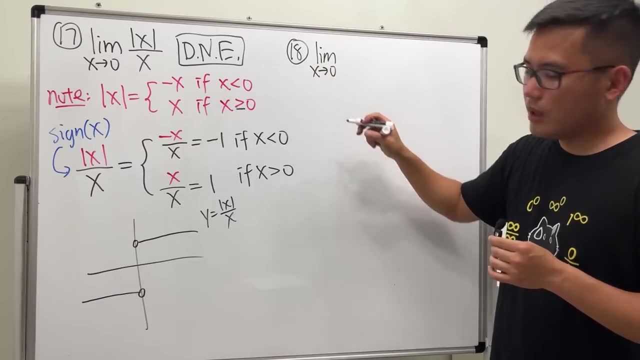 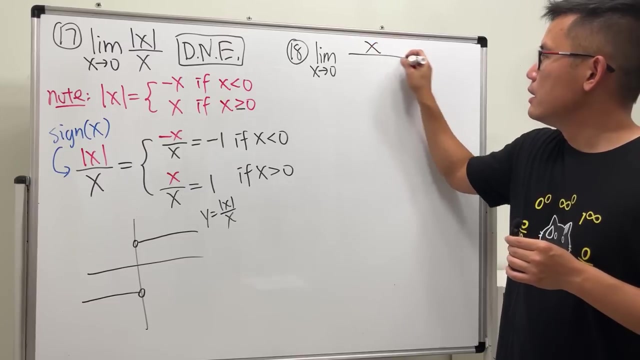 Yay, I think I can run another question right here without erase number 17.. Okay, number 18.. All right, let's take a look at the limit as x approaching zero, and then we have x over absolute value of x plus x squared. 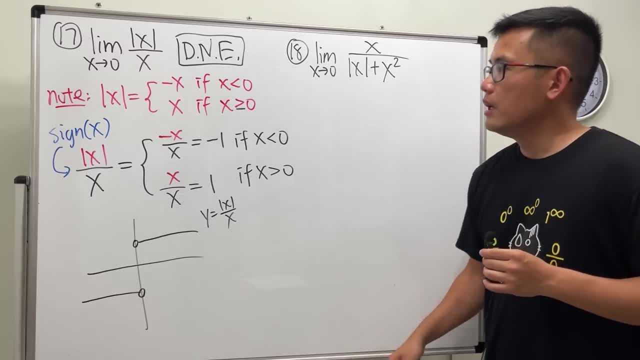 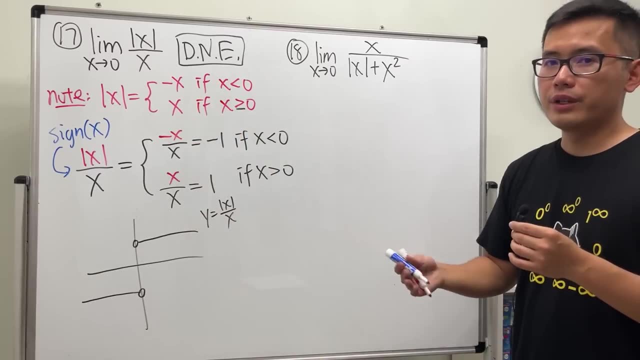 All right. So how can we do this? You can use this again, You can just rewrite everything again, Or right here, let's just go ahead and break down into like a positive and negative and check If we have the limit as x approaching zero minus. 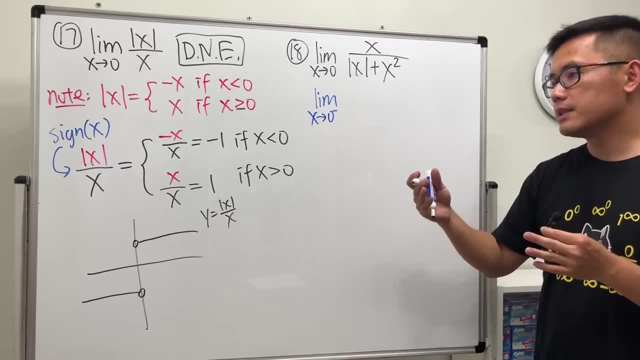 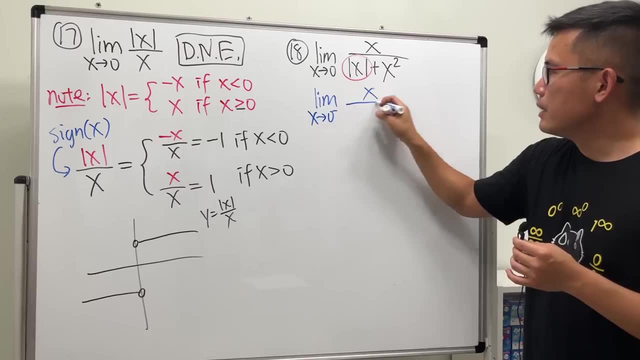 the only thing that's going to. we only have to worry about the following: is this, this part? So x stays, x on the top, but absolute value of x if x is approaching zero minus, meaning the input is negative. this right here. 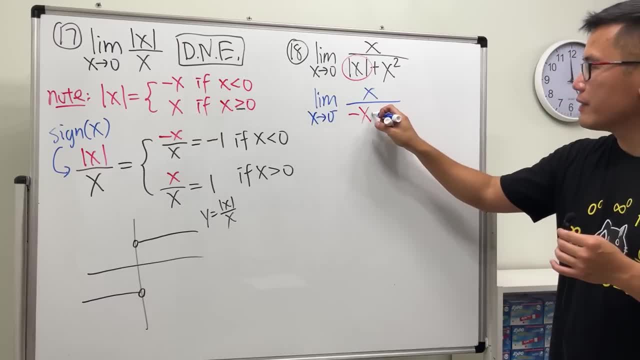 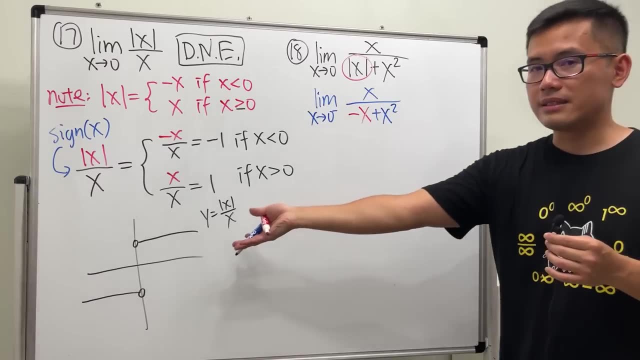 you replace that with negative x, And then right here you have the plus x squared. So that's how you can do it. okay, You could have done the same thing like this earlier, but I think that's more clear. Anyway, once you write this, we can simplify it. 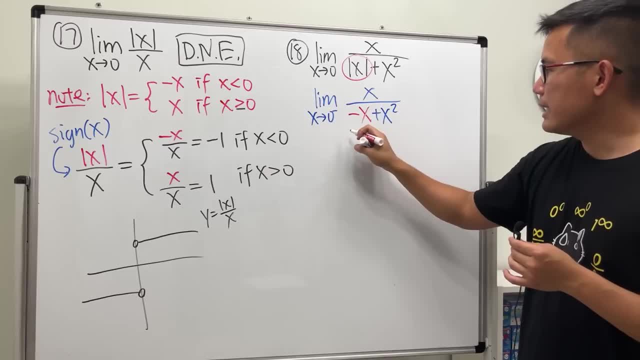 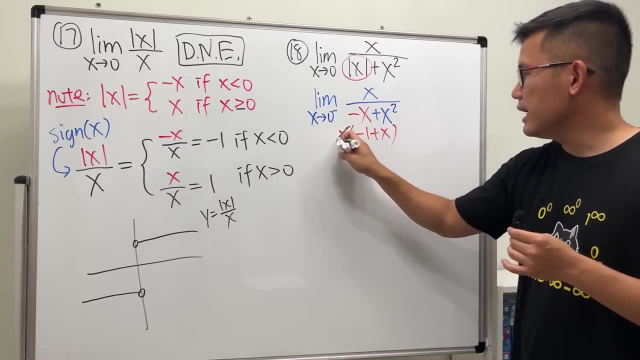 You'll see, on the bottom we can factor on x. So let me do that. and then we have negative one plus x, And then we can see that this x and that x cancel out And that's okay, because when we have x is approaching zero minus. 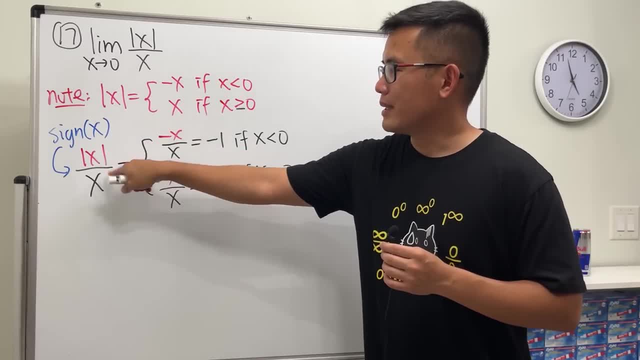 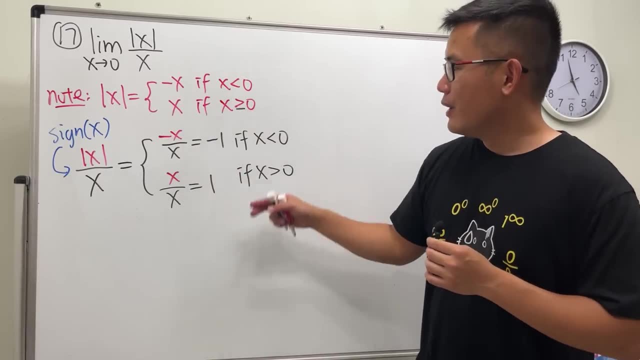 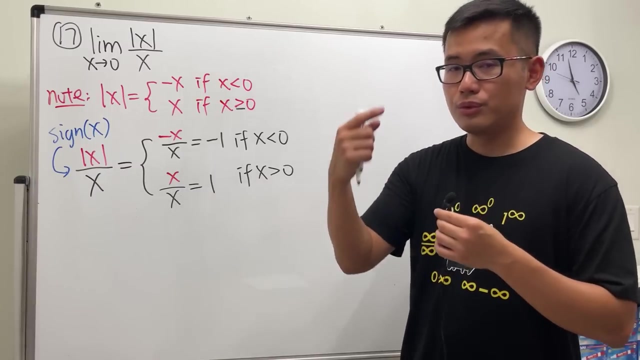 well, i don't know if depends on your teacher, but yeah, but you need to know this and the piecewise function for that. anyway, what's the answer for that? from the negative side, we get negative one. from the right hand side, we get positive one, so they do not equal. you can make a graph of this real quick. 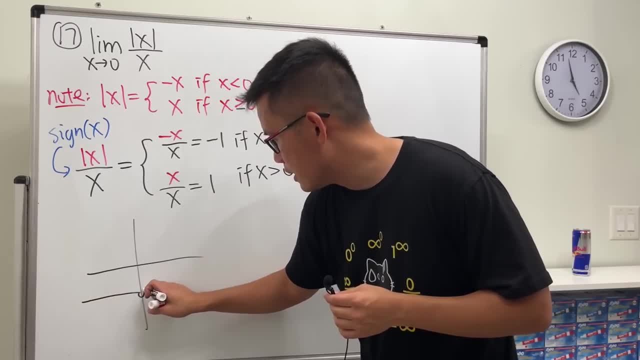 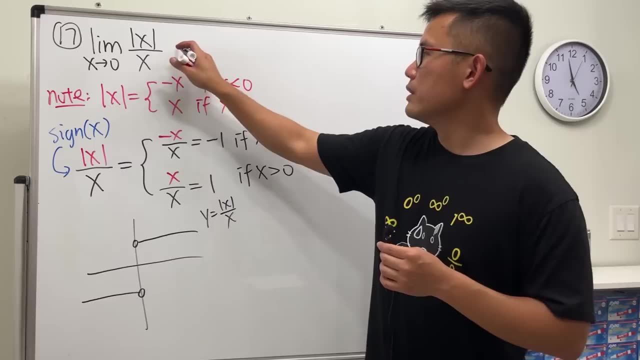 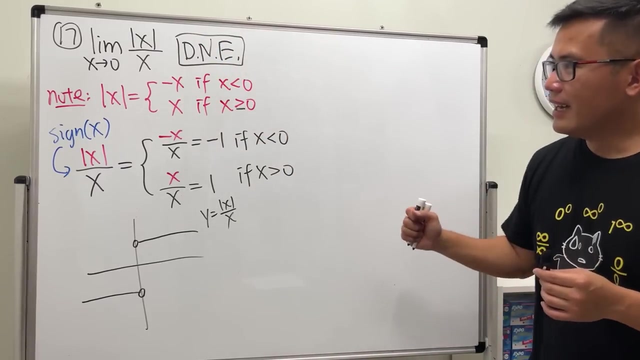 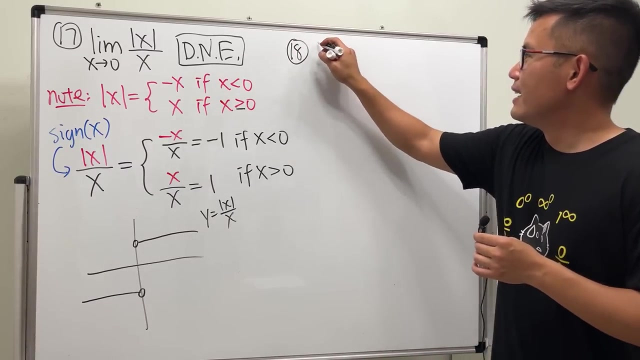 negative one and then one, and this is the graph for absolute four of x over x. but either way, though this right here does not exist. yay, i think i can run another question right here without erase number 17. okay, number 18. all right, let's take a look at the limit as x approaching zero. 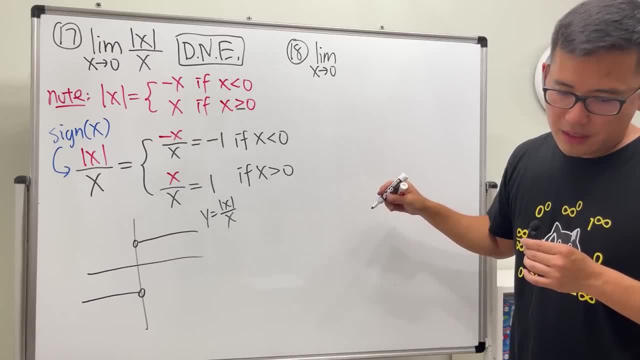 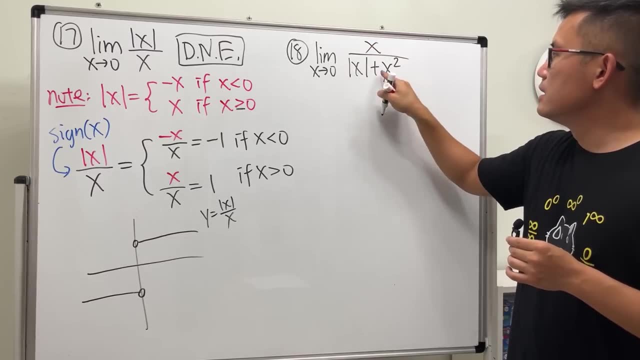 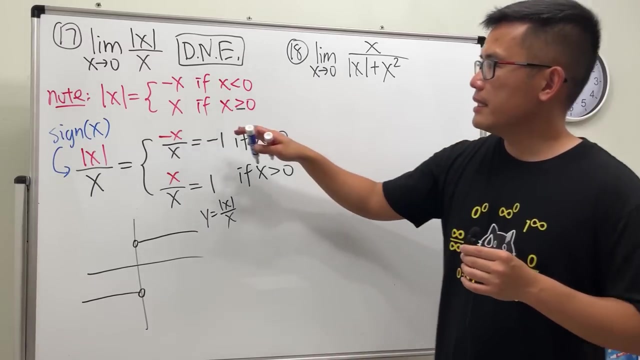 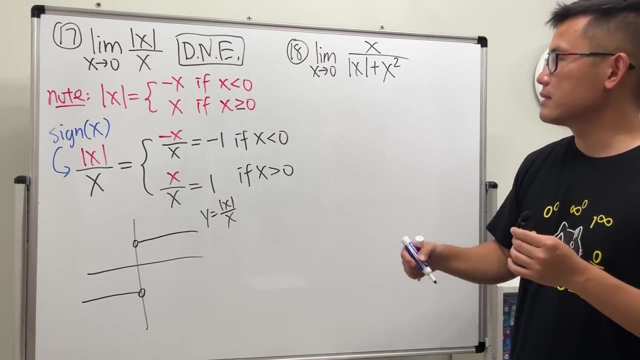 and then we have zero x over absolute four of x plus x square. all right, so how can we do this? you can use this again, you can just rewrite everything again, or right here, let's just go ahead and break down into like a positive and negative and check if we have the limit as x approaching zero. 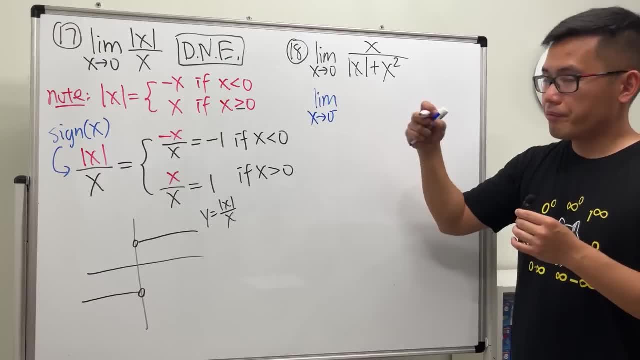 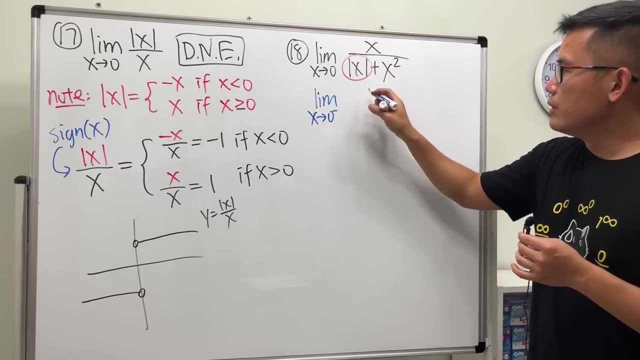 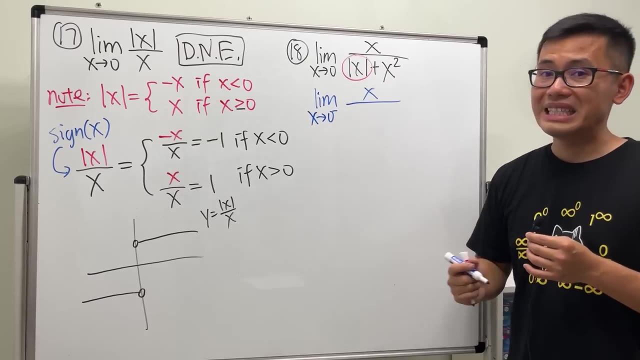 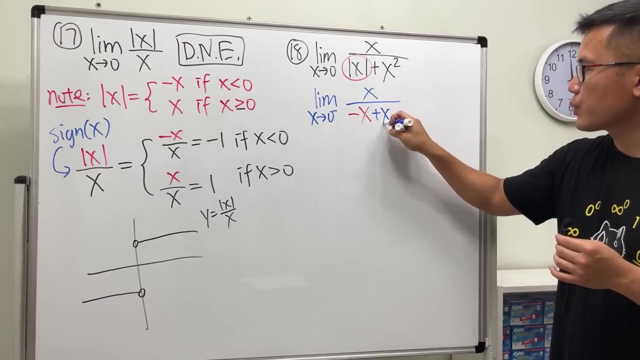 minus. the only thing that's going to- we only have to worry about the following- is this, this part. so x stays, x on the top, but after five x, if x is approaching zero minus, meaning the input is negative, this right here. you replace that with negative x and then, right here, you have the plus x squared. so that's how you can do it, okay, you. 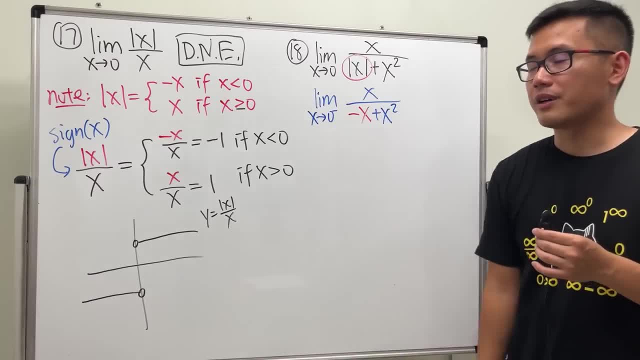 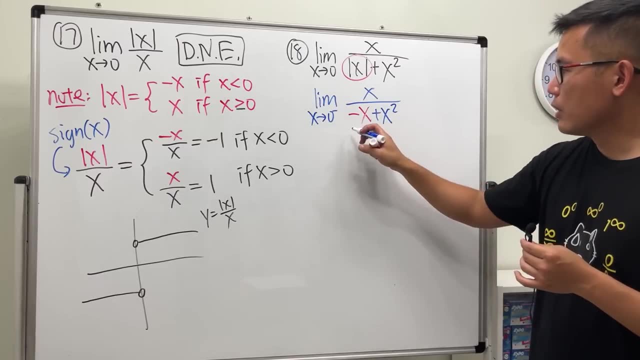 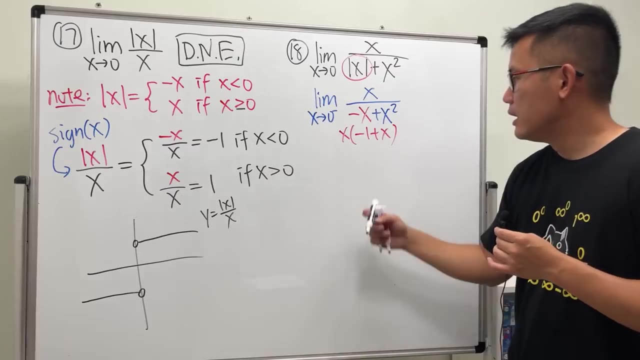 could have done the same thing, like like this earlier, but i think that's more clear. anyway, once you write this, we can simplify it. you see, on the bottom we can factor out an x. so let me do that, and then we have negative 1 plus x, and then we can see that this x and that x cancel out. 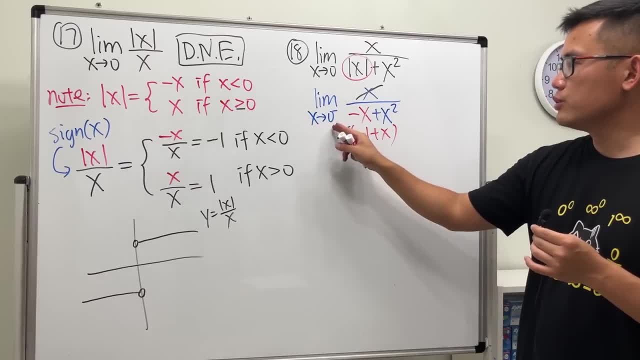 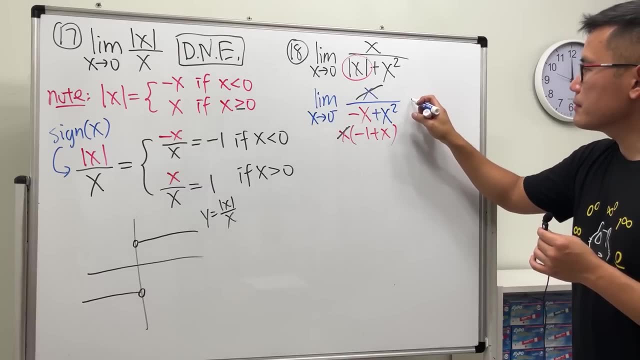 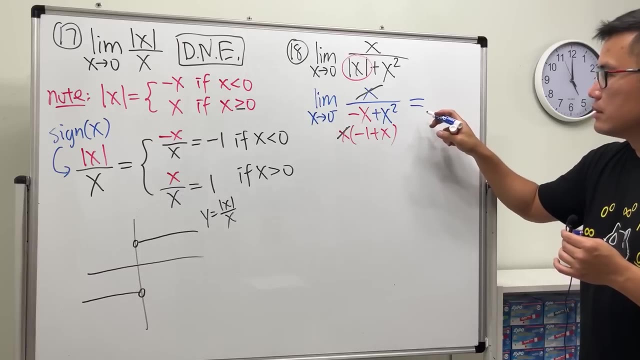 then that's okay, because when we have x is approaching zero minus x is not exactly equal to zero. so cancel it out, that's totally fine, and then we will have what we have: one over negative 1 plus plus x, right? So let's see, Let's just plug in 0 into here, Then we are going to get 1. 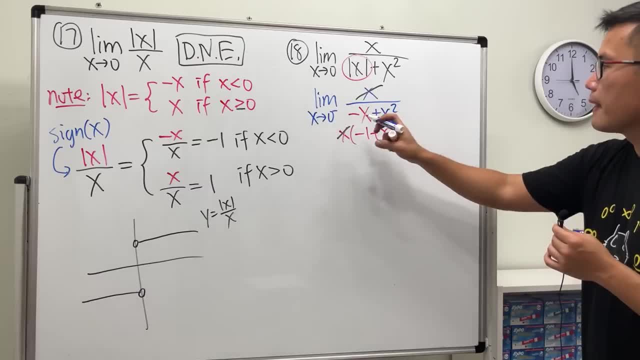 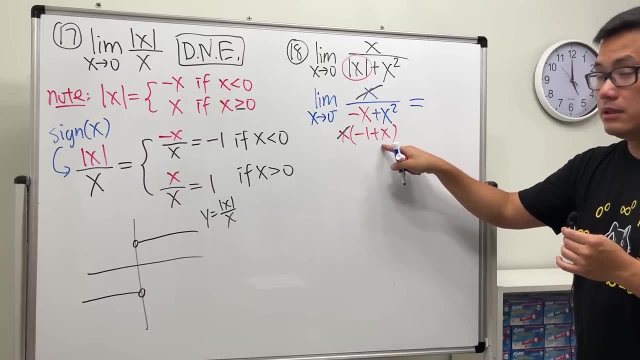 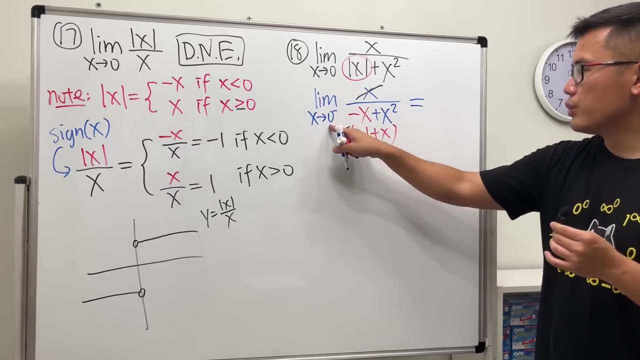 x is not exactly equal to 0, so cancel it out, That's totally fine, And then we will have what We have: 1 over negative, 1 plus x, right? So let's see, Let's just plug in 0 into here. 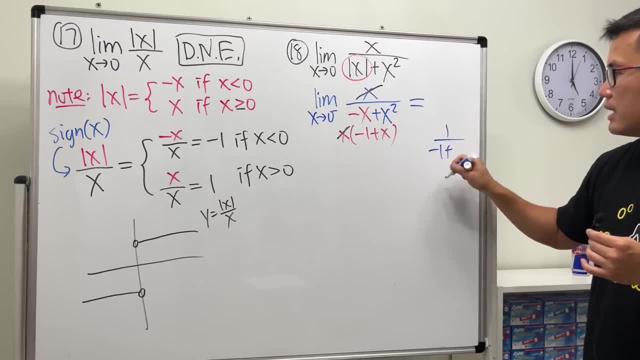 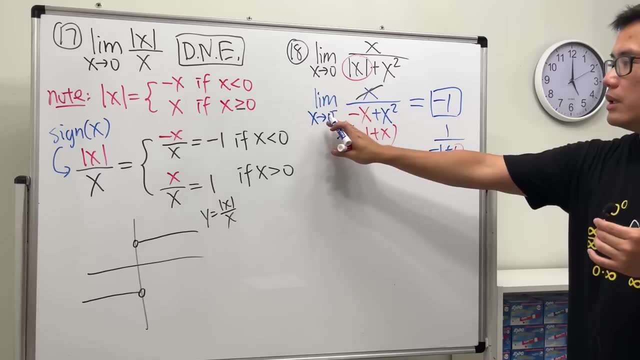 Then we are going to get 1 over negative, 1 plus 0. And we can draw a conclusion right here: The answer is just negative 1. So this limit gives us negative 1.. Similarly, let's do the limit as x approaching 0 plus. 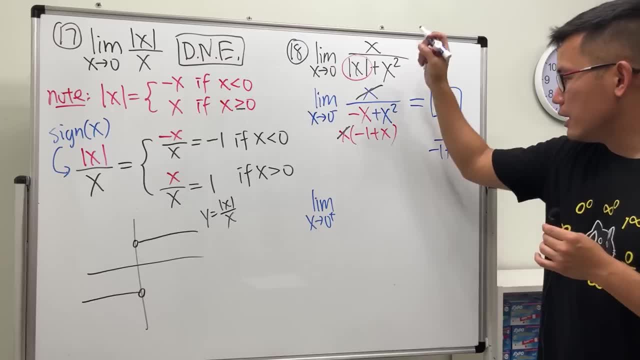 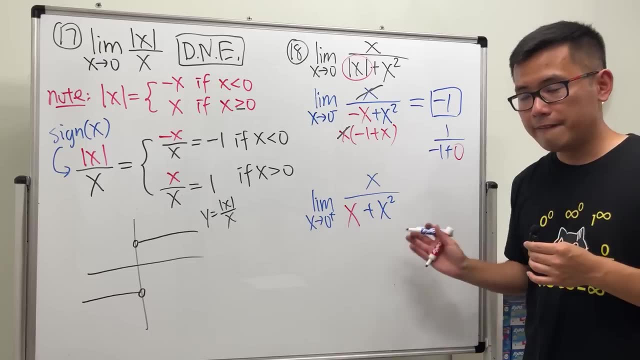 And in that case- again, this is the only part that has to change. On the top is still x, This guy is just x. And then we have plus x squared, Factor out an x on the bottom And then cancel out this x and that x. 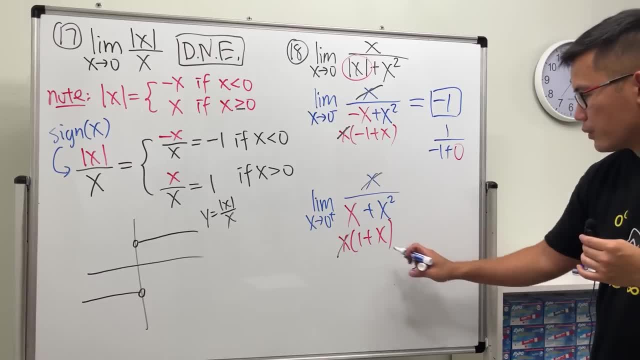 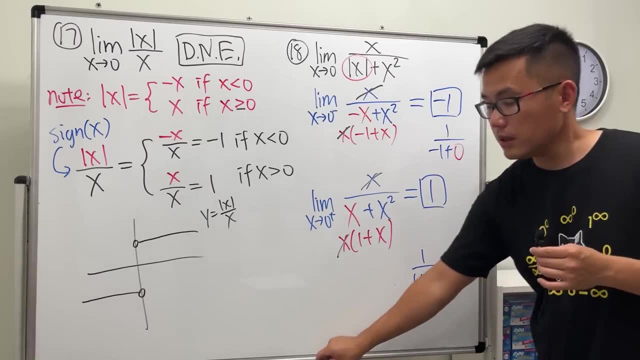 And then put a 0 in here, Then you see we get 1 over 1.. 1 plus 0. And that will give us 1.. So this limit gives us positive 1.. However, 0 minus and 0 plus, they give us different limits. 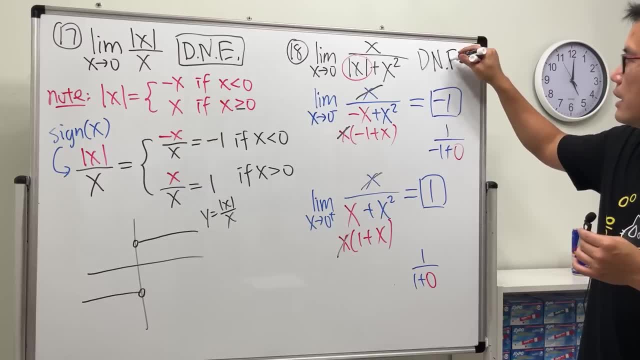 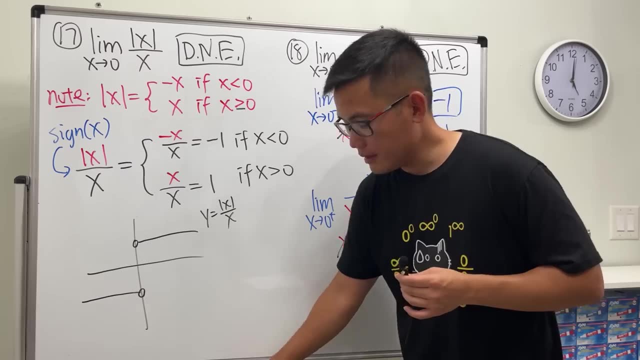 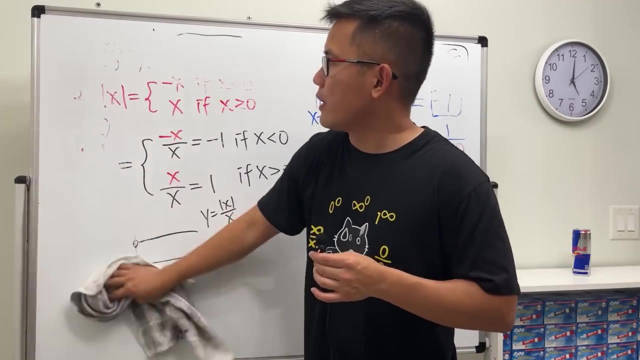 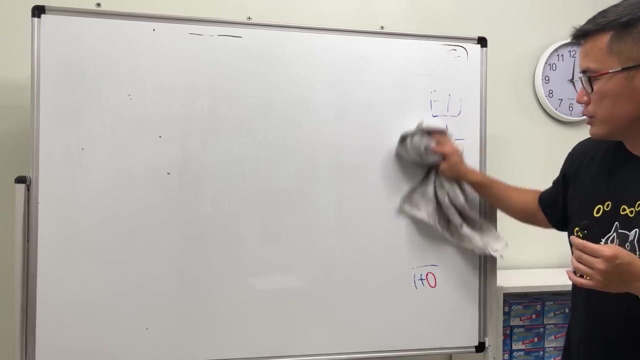 So the answer for this right here does not exist. Okay, Cool. Now another special function for you guys, for number 19.. Namely, the flow. But let me erase the ball first And I'll give you guys a quick intro and then show you guys how to do this. 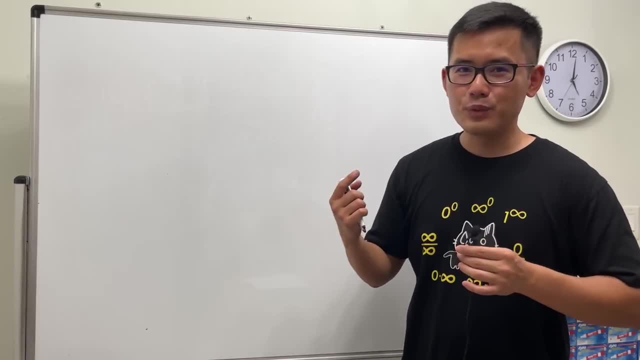 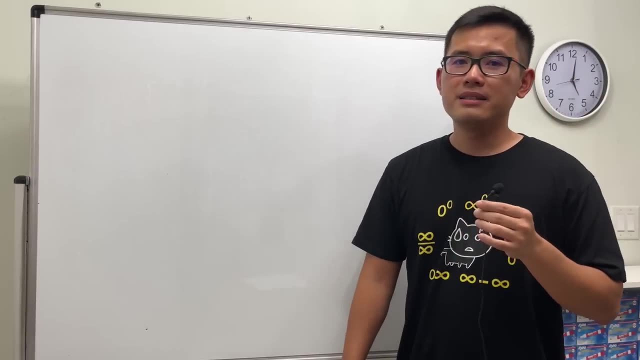 I'm not sure if you guys can see I'm actually sweating, Because right now it's like 5. PM. Yeah, And it's hot And I cannot turn on my AC because one my AC doesn't really work. 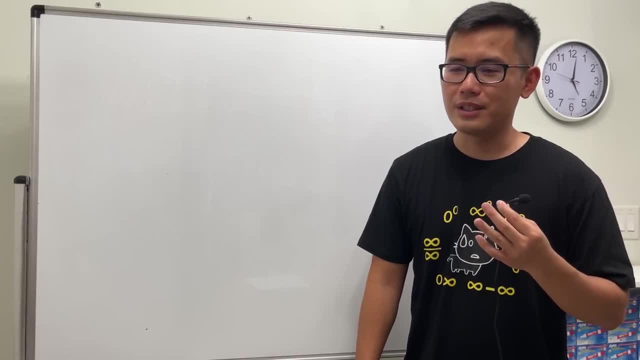 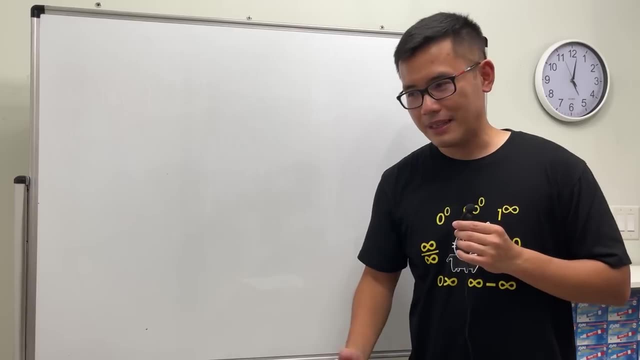 And I should have told you that as reason number one, I cannot really turn on my AC because one, if I turn on my AC, then it will be super loud. That's going to ruin the video. And the second reason is that my AC doesn't really work anyway. 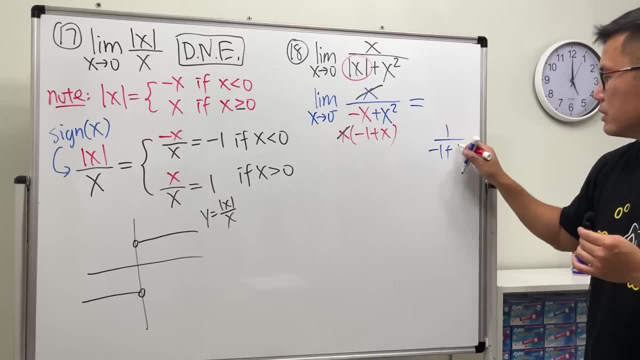 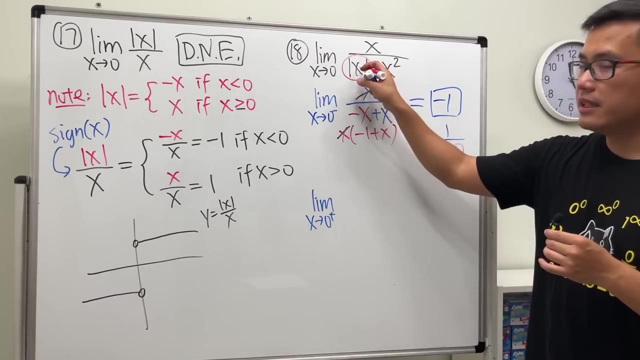 over negative 1 plus 0. And we can draw a conclusion right here. The answer is just negative 1.. So this limit gives us negative 1.. Similarly, let's do the limit as x approaching 0 plus, And in that case, again, this is the only part that has to change. On the top is: 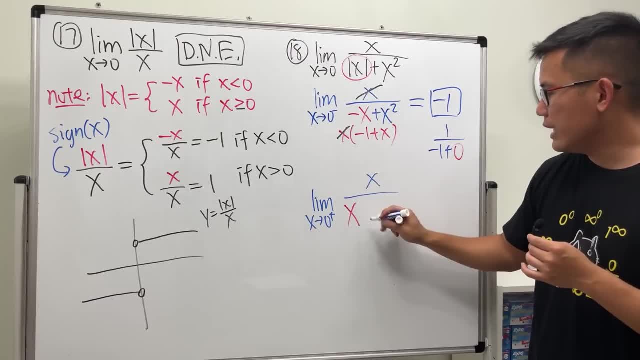 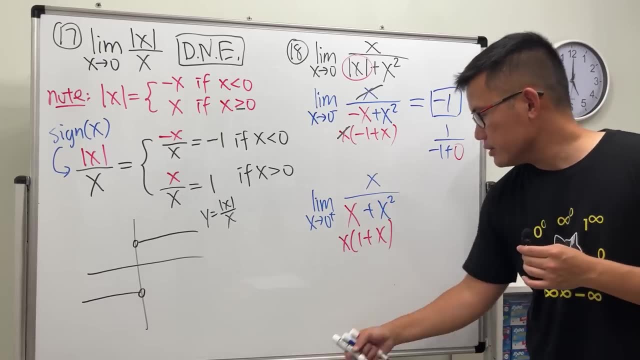 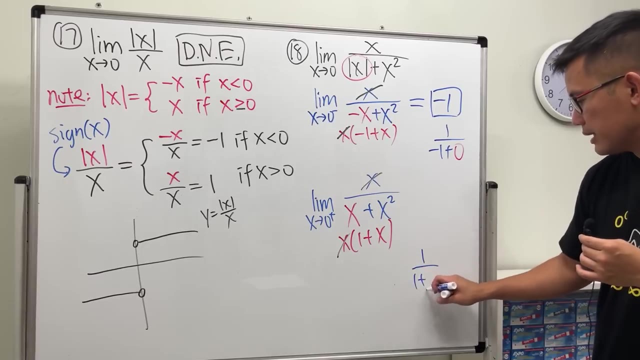 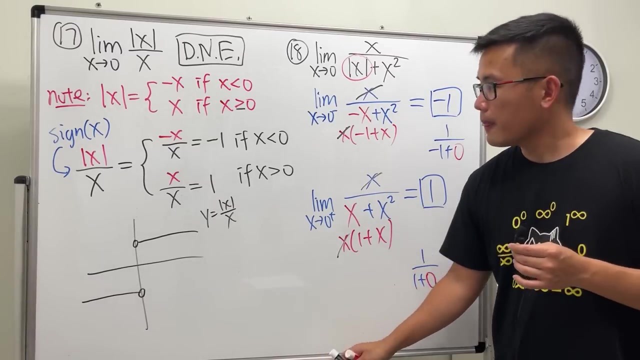 still x. This guy is just x. And then we have plus x squared. Factor out an x on the bottom And then cancel out this x and that x And then put a 0 in here. Then you see we get 1 over 1 plus 0. And that will give us 1.. So this limit gives us positive 1.. However, 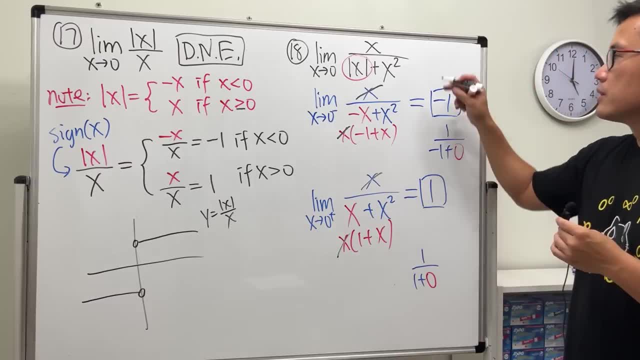 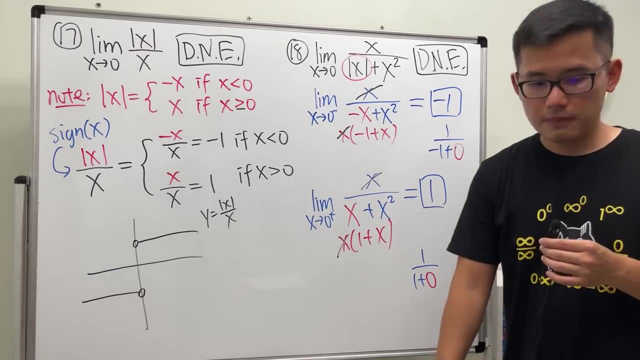 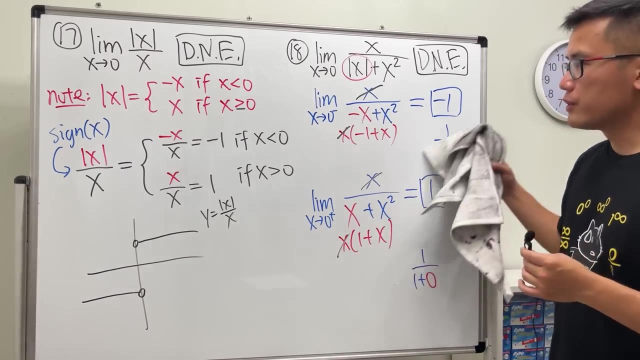 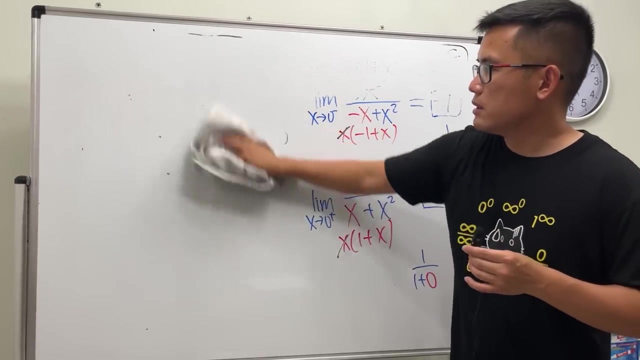 0 minus and 0 plus. they give us different limits, So the answer for this right here does not exist. okay, cool. now another special function for your guys, for number 19, namely the flow function. but let me erase the ball first. I'll give you guys a quick intro and then show you guys how to do this. 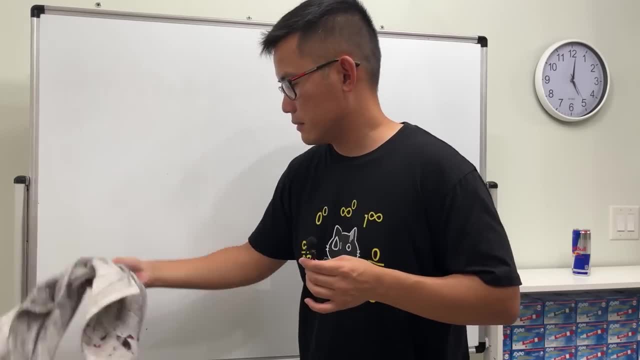 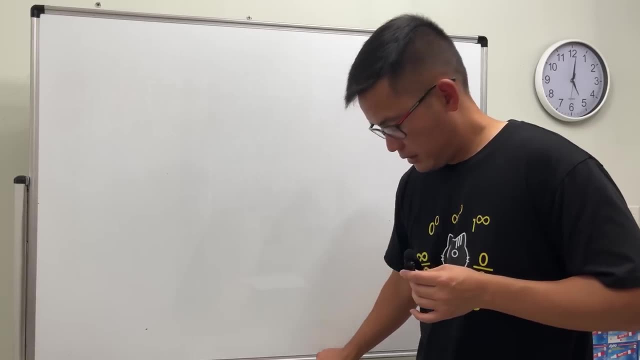 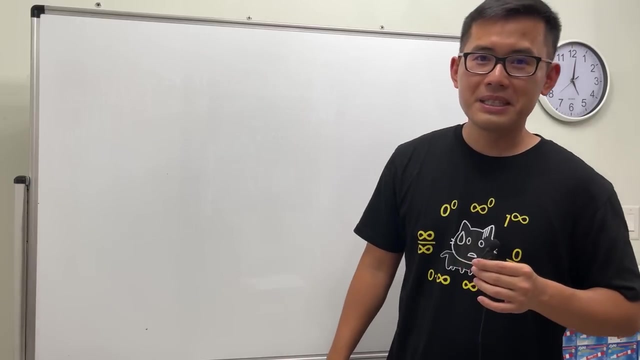 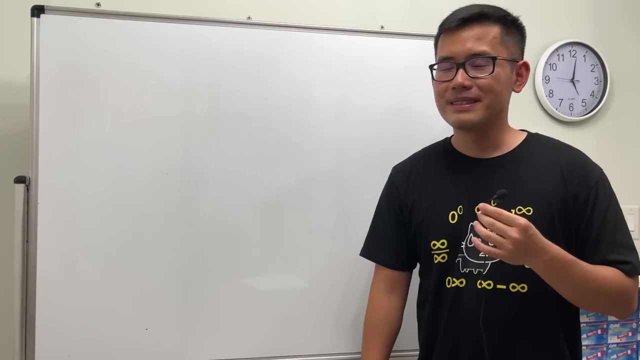 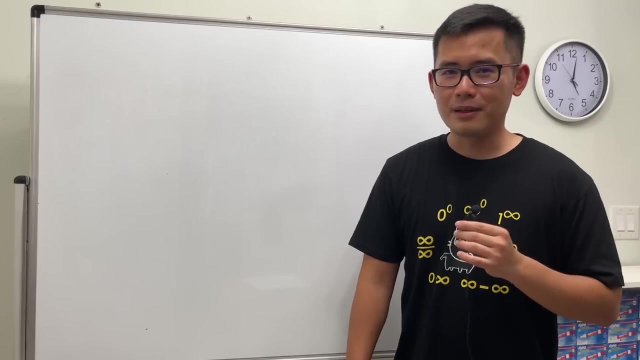 I'm not sure if you guys can see I'm actually sweating because right now it's like 5 pm, yeah, and it's hot and I cannot turn on my AC because one. my AC doesn't really work and I should have turned on my AC because one. if I turn on my AC then it will be super loud. that's going to ruin. 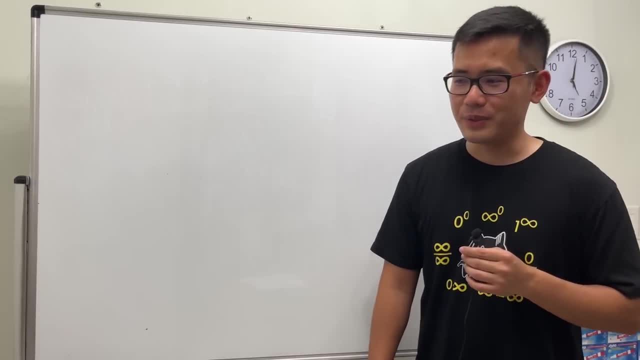 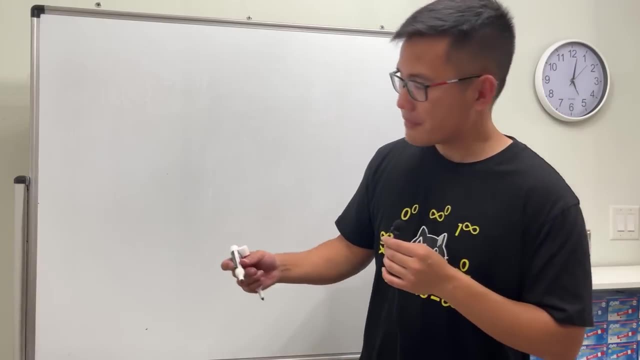 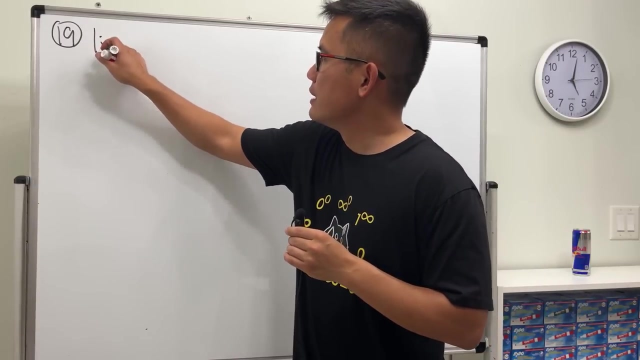 the video. and the second reason is that my AC doesn't really work anyway, but it will be loud. that's the main question. that's the main issue, though, anyway, number 19.. okay, here is the limit as x approaching three. and then, ladies and gentlemen, this is the flow function. 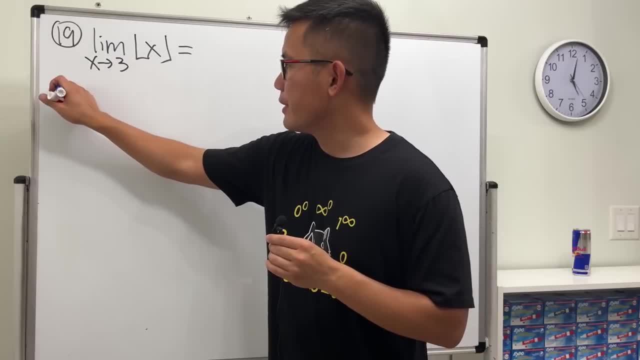 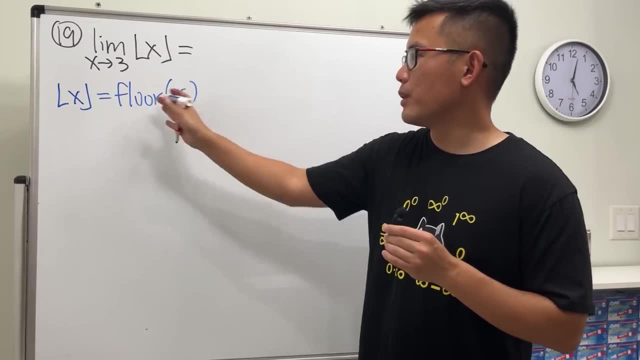 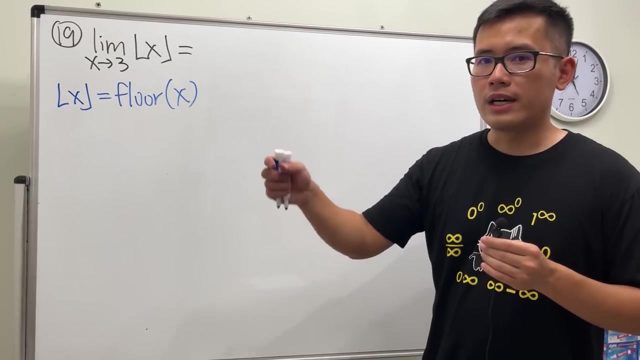 so? so let me explain to you guys what this is. this right here, right, this right here. it's called the fluid function, or some people, like the, will write it as flu of x one way or the other. so what this means is that you just always run down to the. 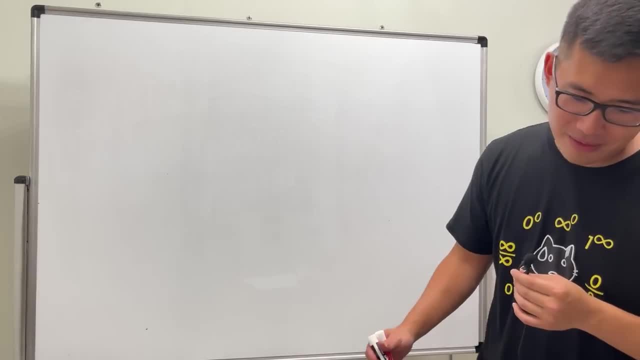 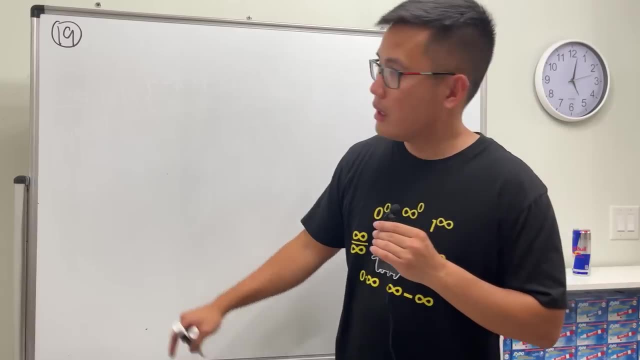 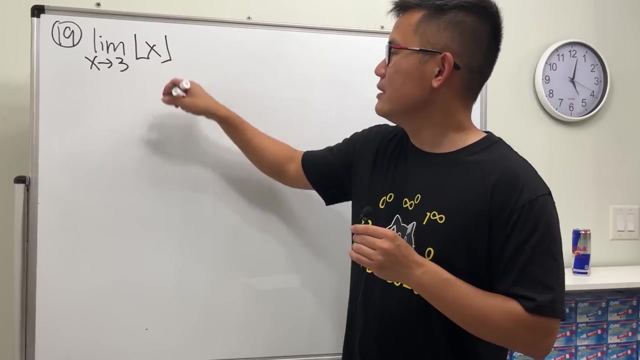 But it will be loud. That's the main question. That's the main issue, though. Anyway, Number 19.. Okay, Here is the limit as x approaching 3.. And then, ladies and gentlemen, this is the flow function. 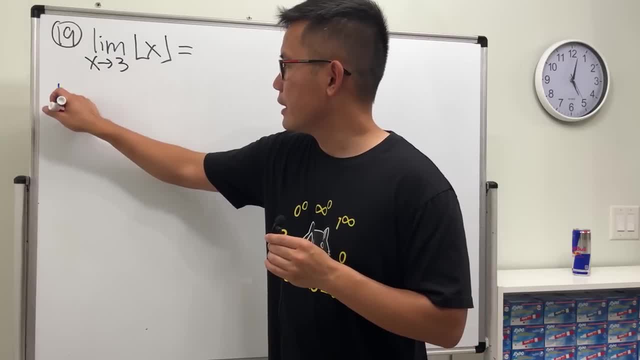 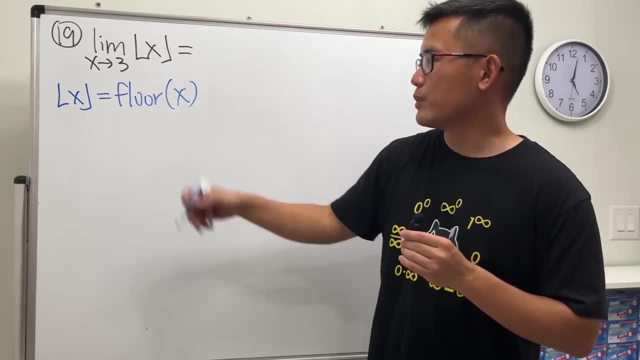 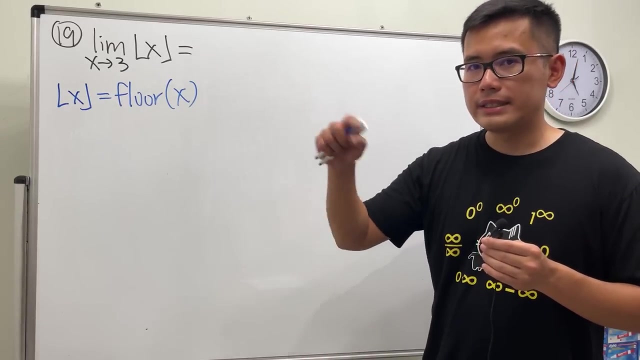 So let me explain to you guys what this is. This right here, All right, This right here. It's called the flow function, or some people will write it as flow of x, one way or the other, And what this means is that you just always run down to the integer: run down. 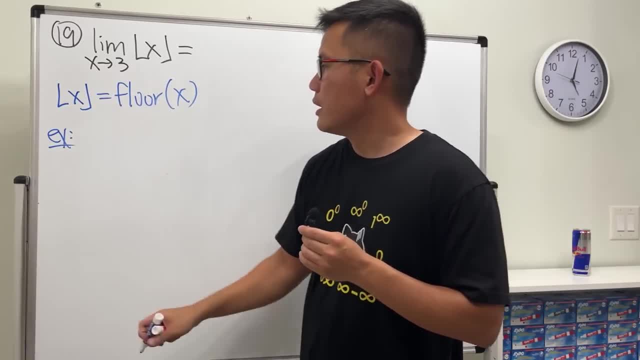 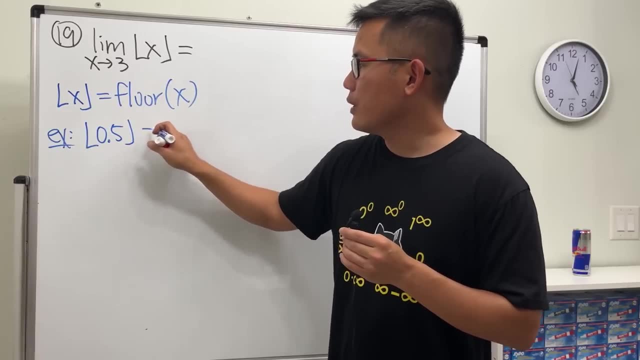 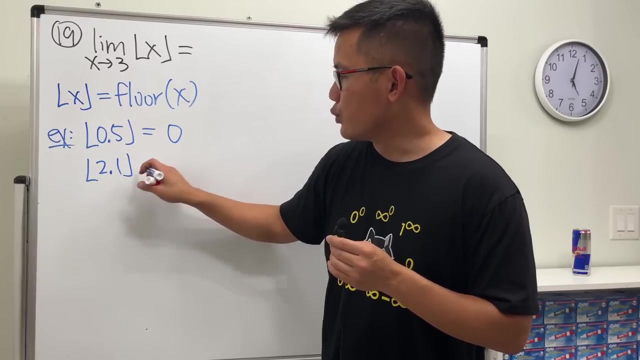 So let me give you an example. When we have the flow of, let's say, 0.5, well, you run down. So this right here will be 0.. Okay, If you have flow of 2.1, you run down. 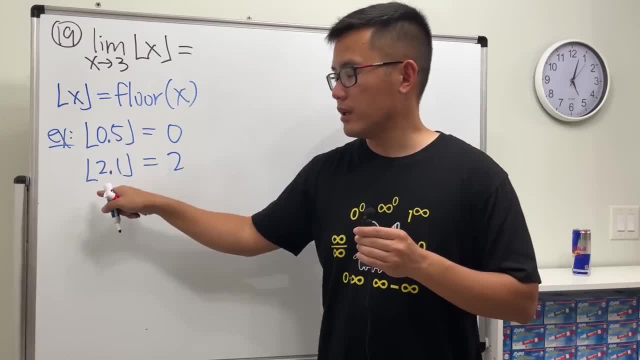 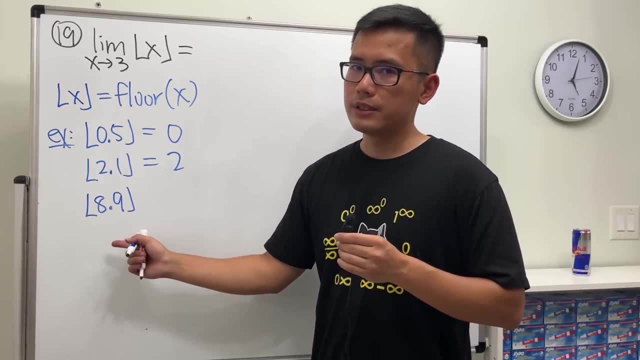 So this is going to be 2. Right, You run down to the integer And then, if you have the flow of, let's say, 8.9, man, this is almost 9,. right, But no, you still run down. 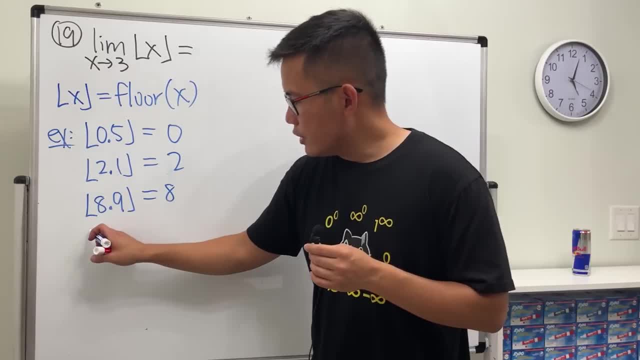 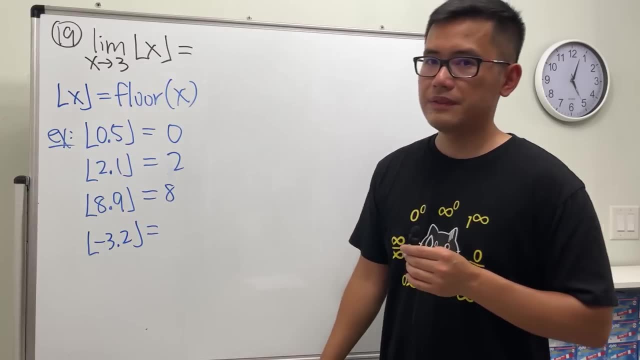 So this right here is equal to 8.. And it might be a little bit trickier if we have negative numbers, such as negative 3.2.. What's the answer for this? It's not negative 3, but rather it's negative 4.. 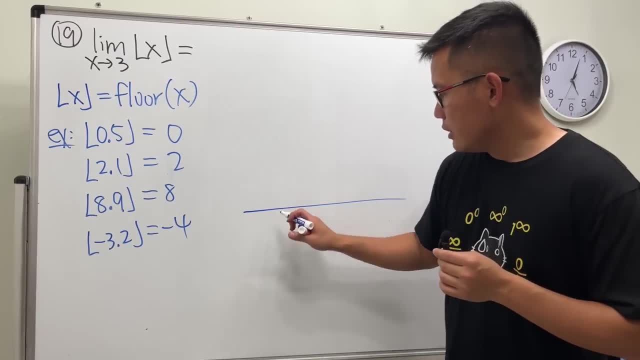 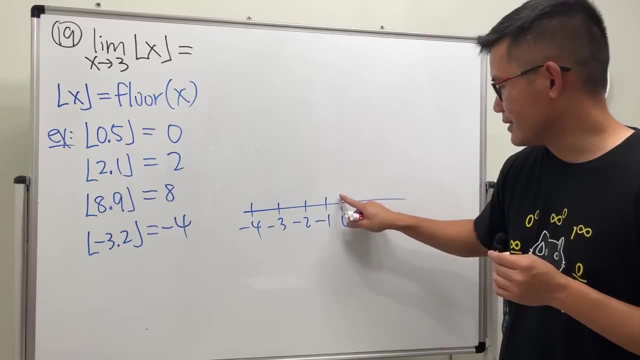 Perhaps the easier way to see is on the number line. Okay, So you have the 0 and then negative 1,, negative 2,, negative 3, and negative 4, right, I know this is like a horrible picture. Much better. 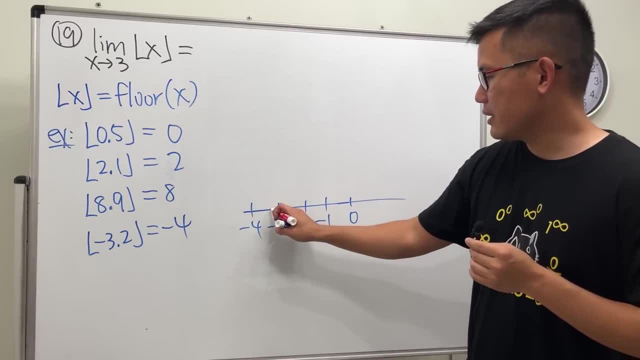 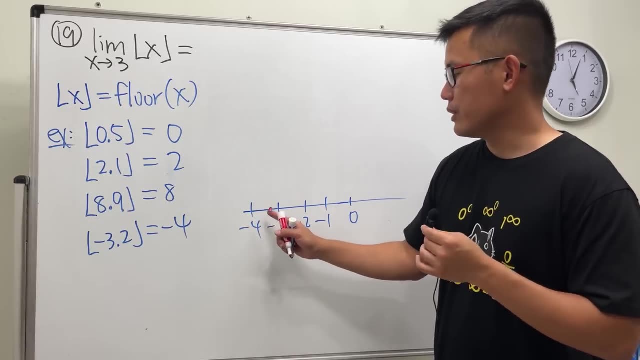 Negative 0.. Sorry, negative 3.2 is right here And you always run down, So you always move the point to the left, whole number. Well, you just move the, you just run down, and then it's the first integer. 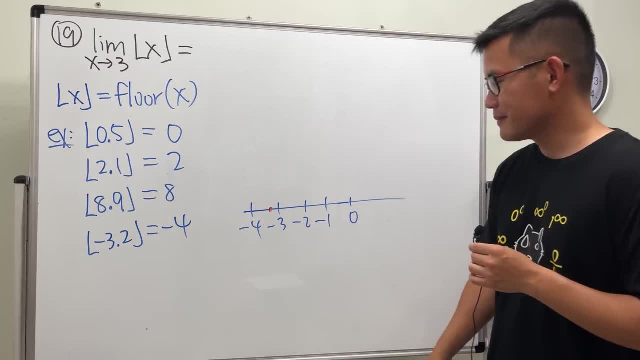 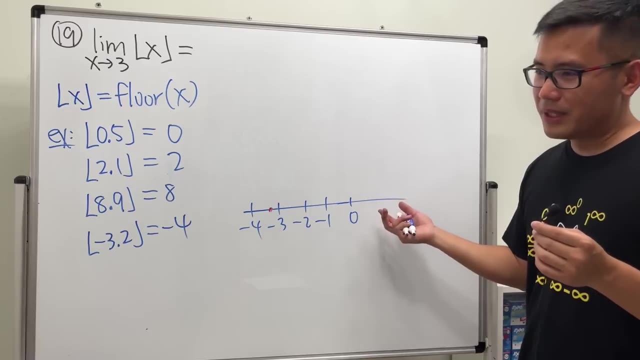 Okay, So you run down. So that's why it's negative. 4. You see that prepared Ripple there. I don't know if I need to drink it, but if I need to I will. It's been an hour, It's hot. 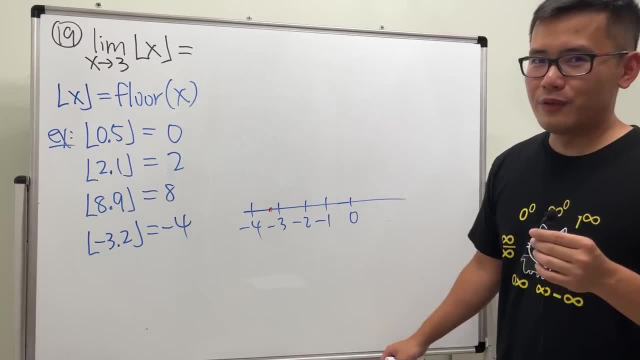 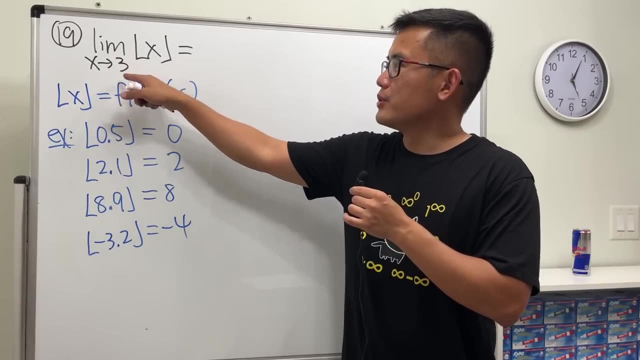 Most likely it's room temperature already. Maybe I'll get one from the fridge, We'll see, But anyway, hopefully this right here is clear. Now, what's the limit as x approaching 3 of the flow function of x? This question will be so much easier if we look at the picture, right. 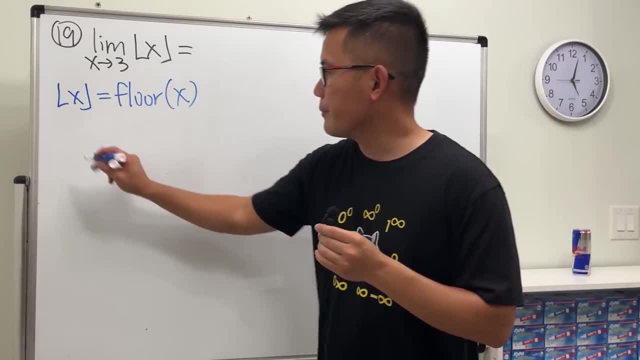 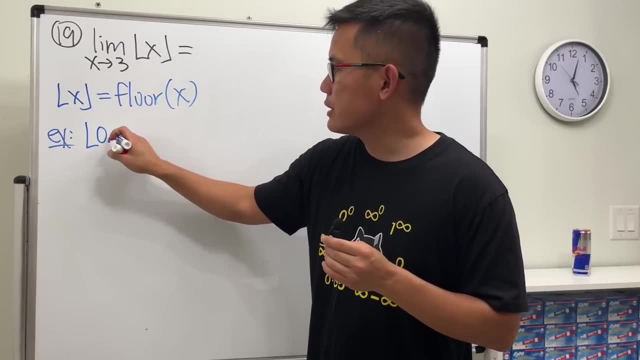 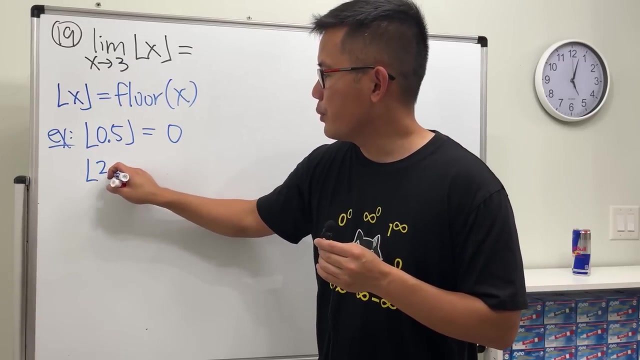 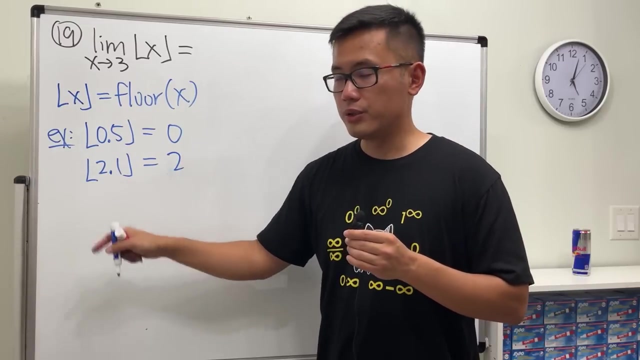 integer right run down. so let me give you an example. when we have the flow of, let's say, 0.5, well, you run down. so this right here will be zero. okay, if you have flow of 2.1, you run down. so this is going to be two right run down to the integer. and then, if you have the flow of, let's say 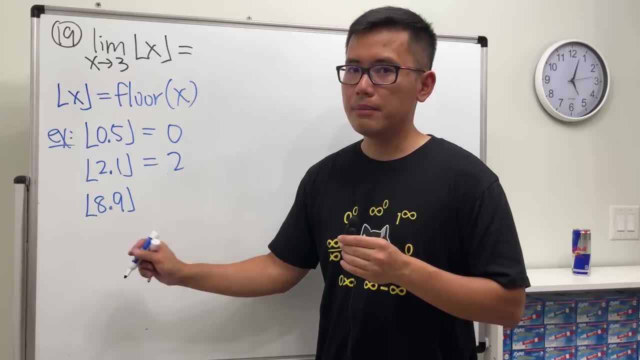 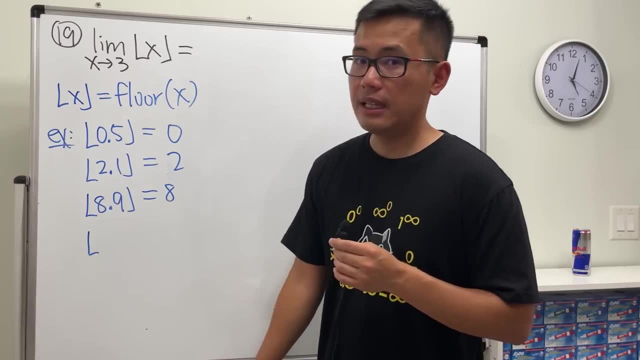 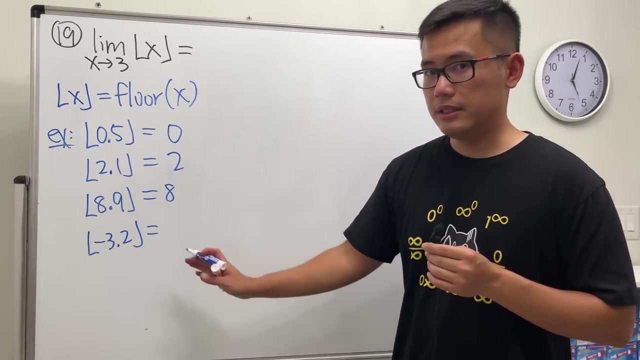 8.9. man, this is almost night, right, but no, you still round down. so this right here is equal to eight, and it might be a little bit trickier if we have negative numbers, such as negative three point two. what's the answer for this? it's not negative three, but rather. 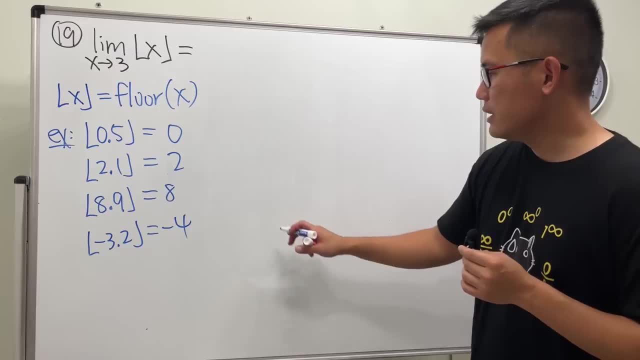 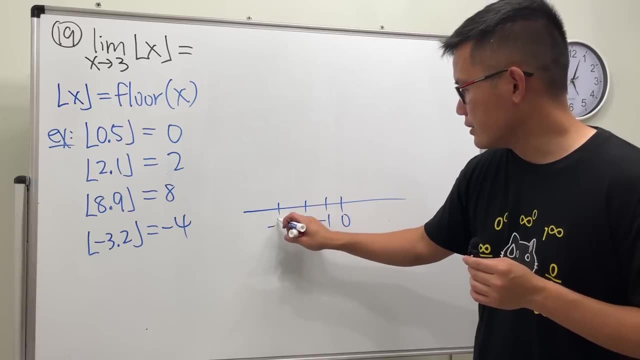 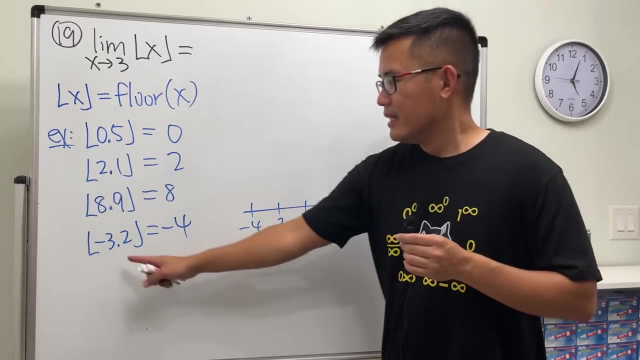 it's negative four. perhaps the easier way to see is that on the number line. so you have the zero and then negative one, negative two, negative three and negative four. right, i know, this is like a horrible picture. much better negative zero points. so negative 3.2 is right here and you always run. 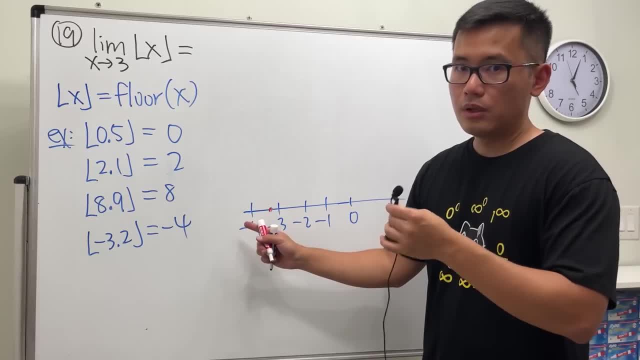 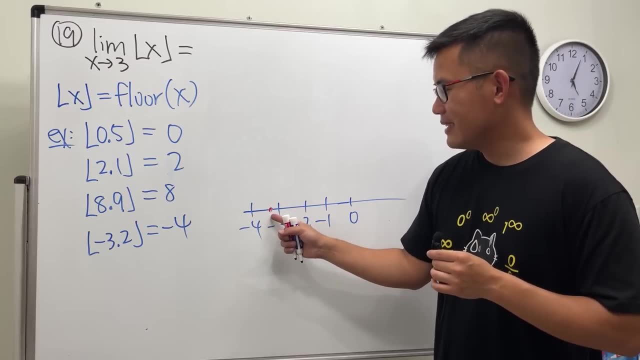 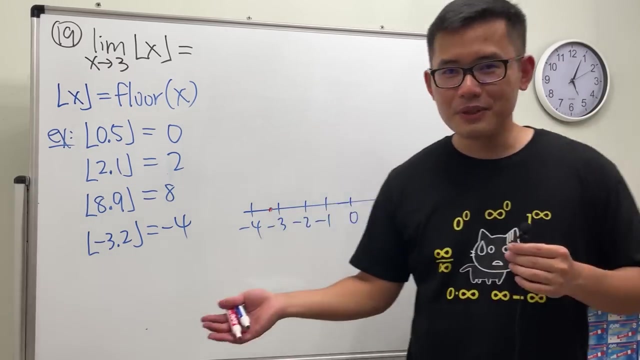 down. so you always move the point to the left whole number. well, you just move that, you just run down. and then it's the first integer, so you run down. so that's why it's negative four. you see that prepared ripple there. i don't know if i need to drink it, but 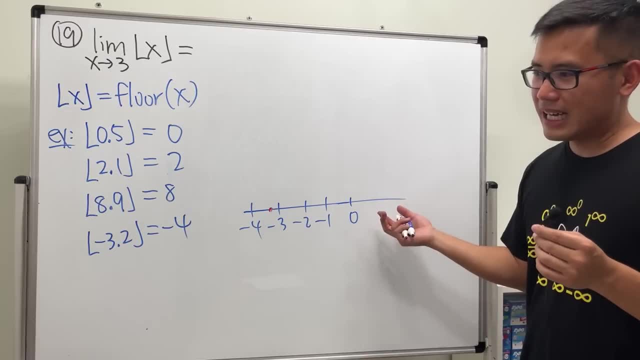 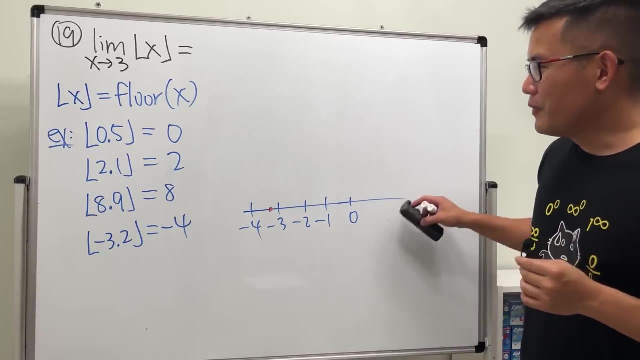 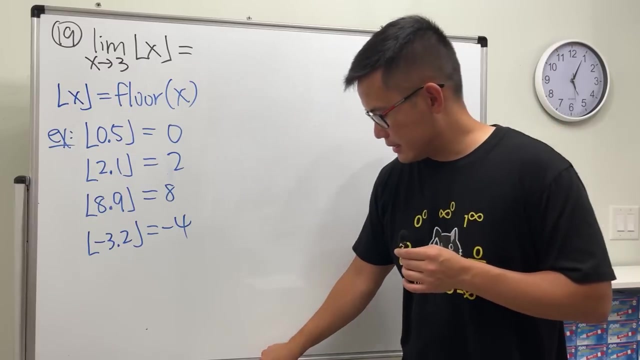 if i need to, i will. it's been an hour, it's hot. most likely it's room temperature already. maybe i'll get one from the fridge, we'll see. but anyway, hopefully this right here is clear now. what's the limit, as x approaching 3, of the fluid function of x? this question will be so much easier if we look at the. 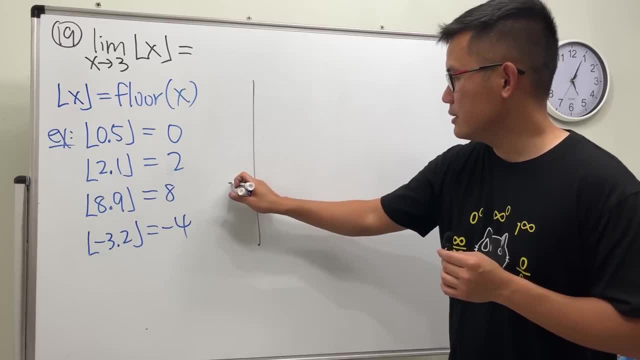 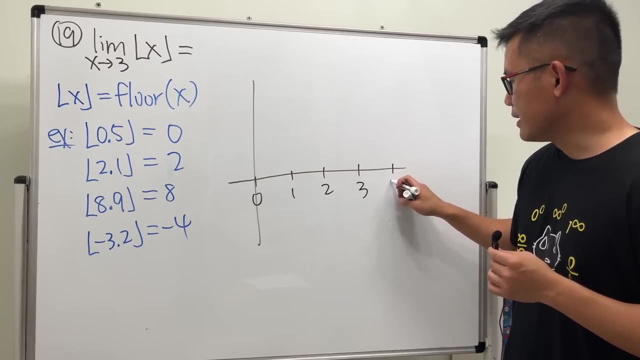 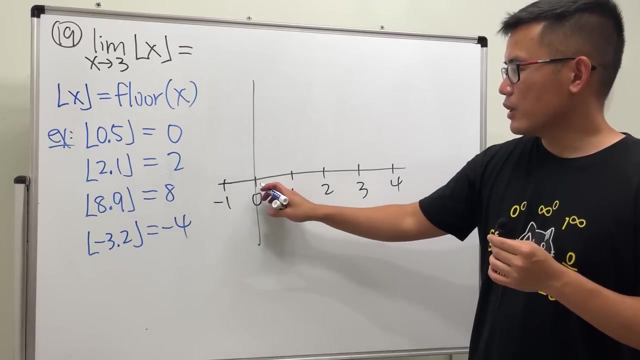 picture. right, so we will look at a picture. ladies and gentlemen, let's have a look. here is 0, 1, 2, 3, minus. well, 4 and minus will let's put negative 1.. so use the id earlier. check this out when x is. 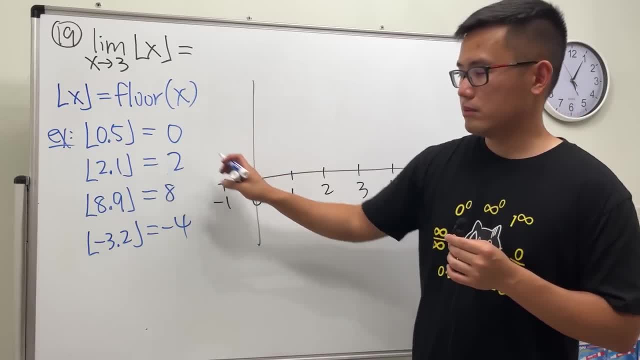 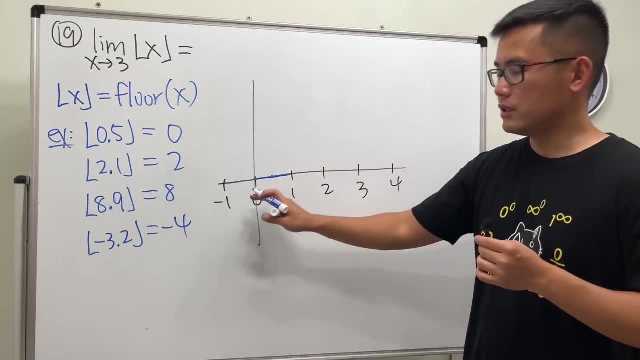 let's say 0.5, the y value will be 0.. when x is 0.9, the y file is still 0.. so, in fact, anything from here to here is just 0. so that's the first piece. however, when we have the app, the flow of 1. 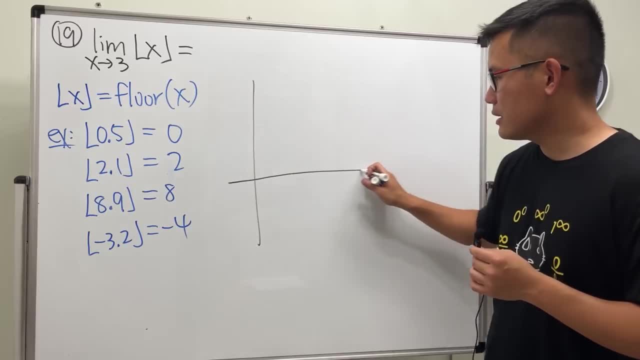 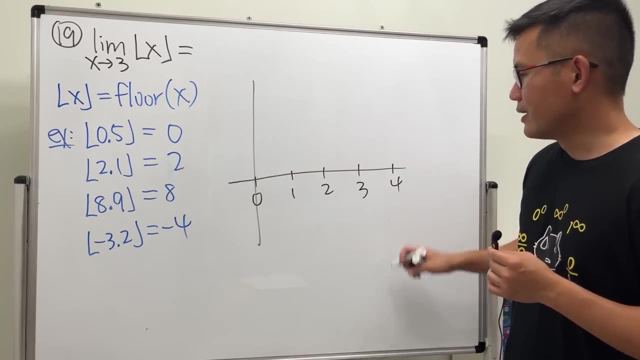 So we will look at a picture, Ladies and gentlemen, let's have a look. Here is 0,, 1,, 2,, 3,, might as well, 4.. And might as well let's put negative: 1.. So use the idea earlier. 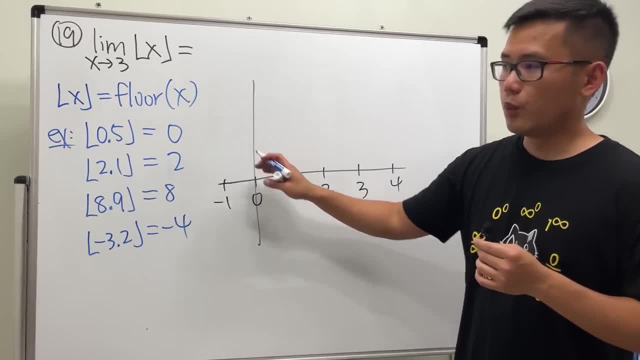 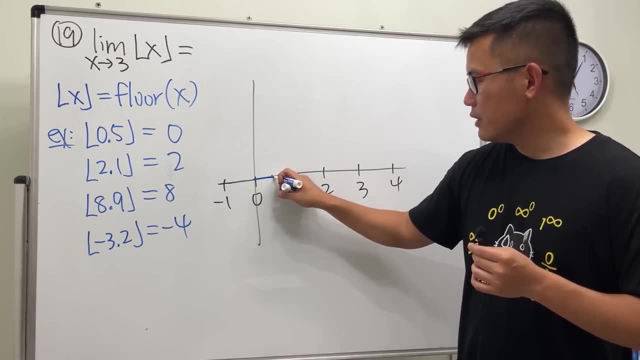 Check this out: When x is, let's say, 0.5, the y value will be 0. When x is 0.9, the y value is still 0. So, in fact, anything from here to here is just 0.. 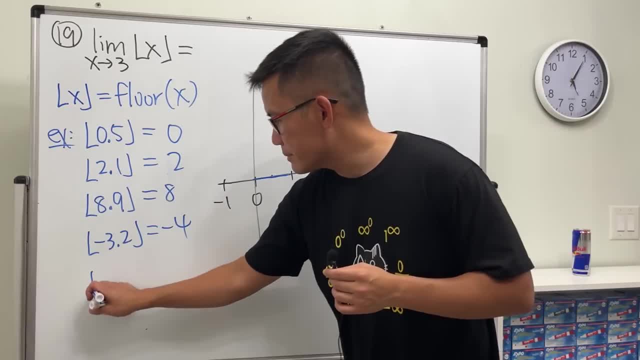 So that's the first piece. However, when we have 0.9,, the y value is still 0. So, in fact, anything from here to here is just 0. So we're going to interrupt this, because it's literally still 0.. 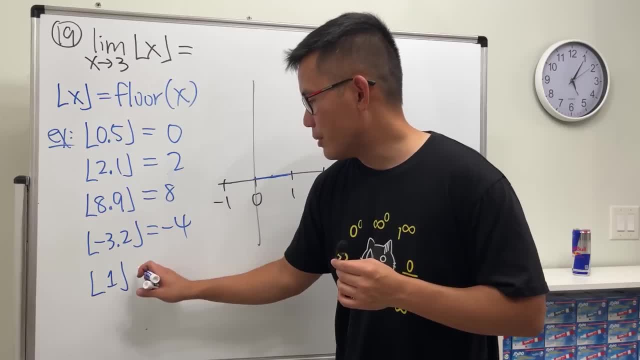 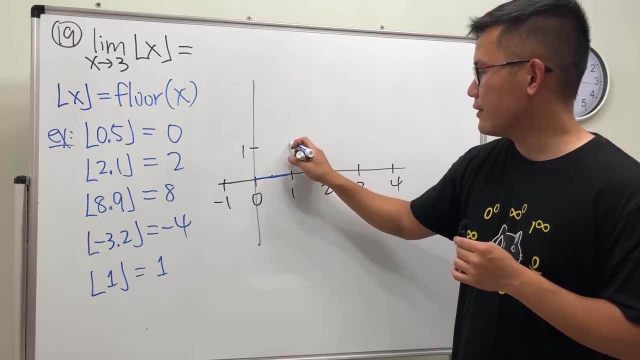 So, for example, let's say that we have the flow of 1.. If this is a whole number already, then you just get the whole number back. So when x is 1, you jump to 1. So you have a closed circle here and you have an open circle here. 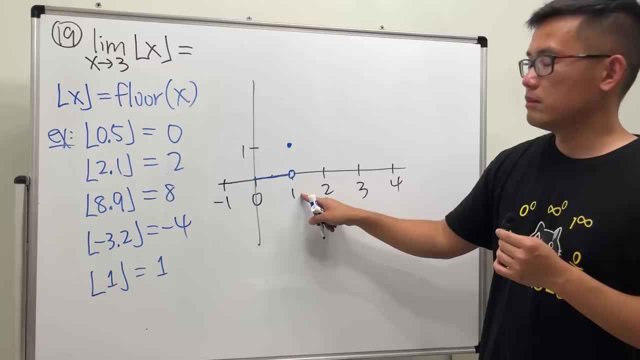 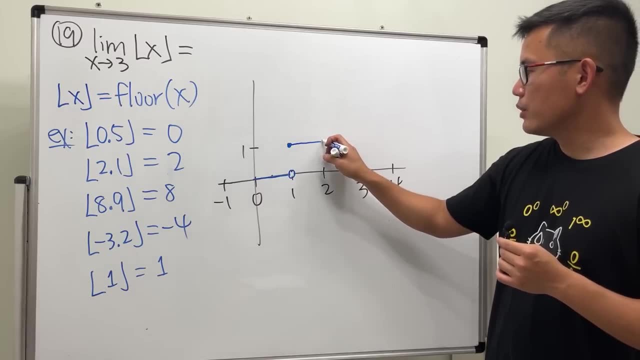 And then you continue. When we have 1.1, the flow of that is 1.. Likewise anything up to almost 2.. Because when x is exactly 2, you make another jump to 2.. Same thing, Okay. 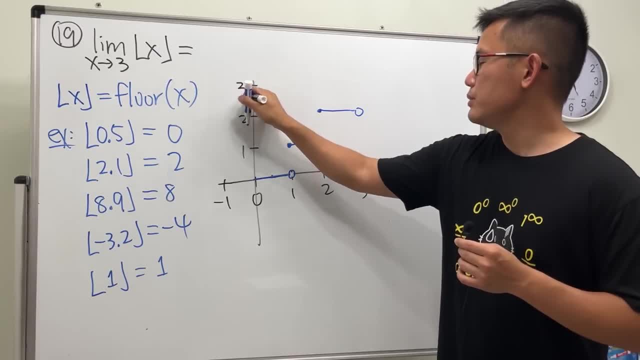 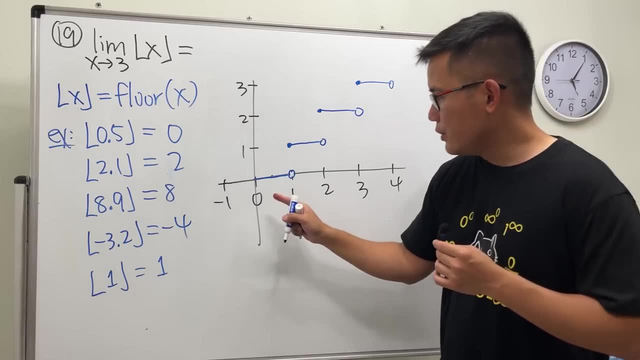 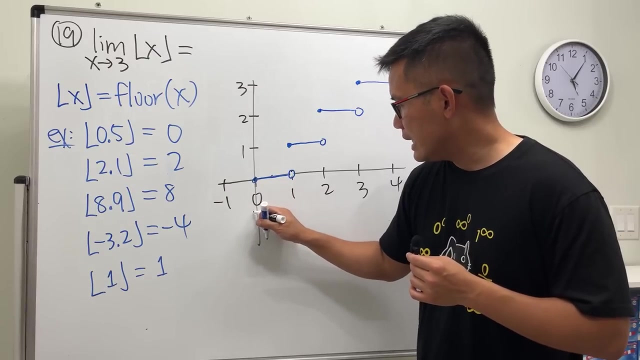 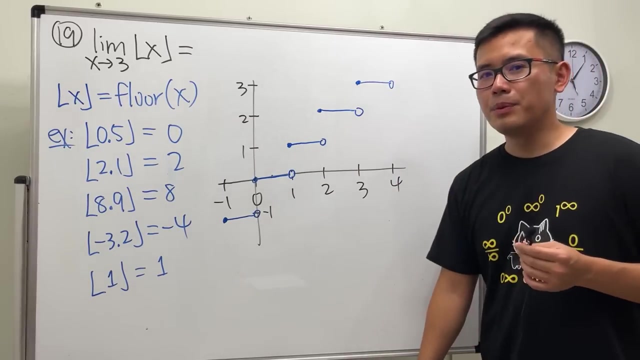 open and then up three and then here and then like this, and then so on, so on, and, if you would like, when x is zero you get zero, and then anything from negative one to here we get negative one, so you have a piece like this. so it's like a stair. i believe some people also call this. 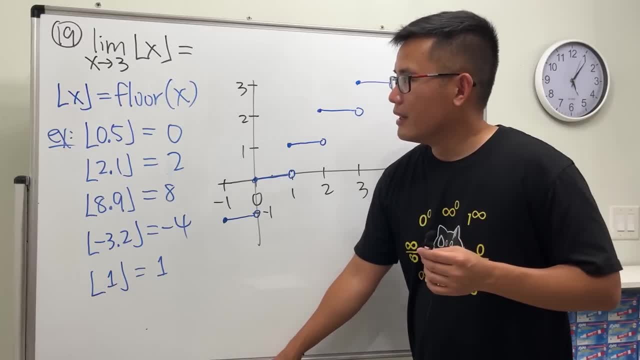 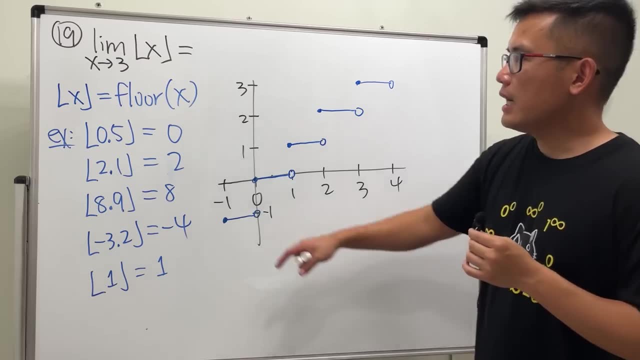 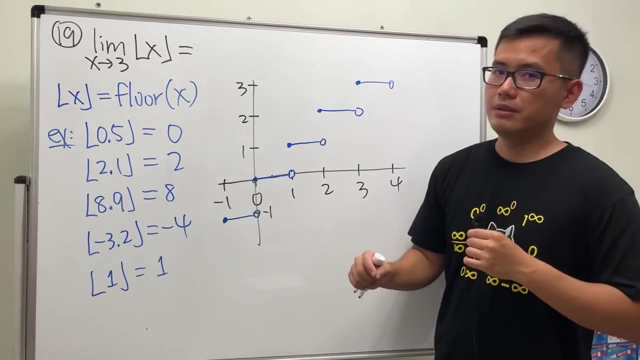 the stair function but, like the flow function, is the most common one, or maybe the greatest integer function. but anyway, though, check this out: when x is approaching three from the left we get two, from the right we get three. so the answer for this right here is: doesn't. 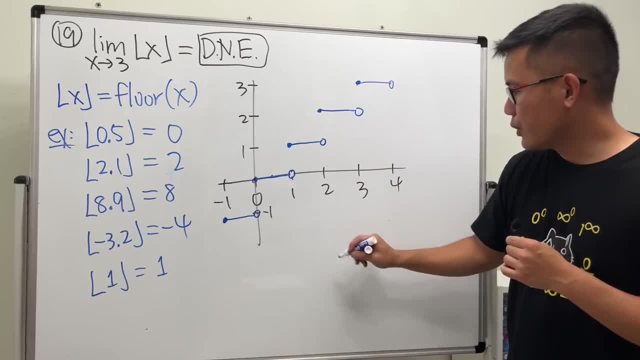 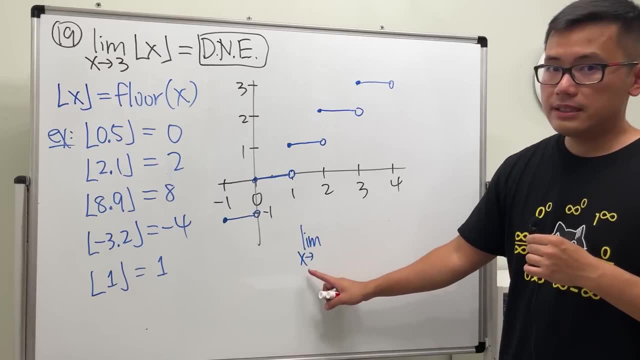 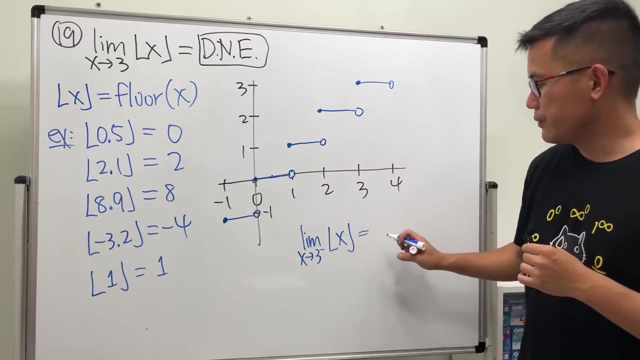 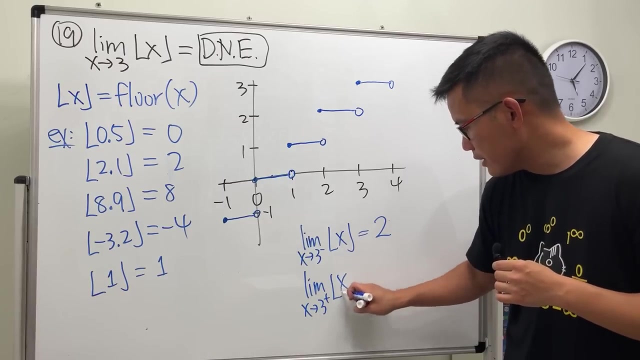 exist. and let me just indicate that real quick. if we have the limit as x approaching two, so if we have the limit as x approaching three from the left hand side, so three minus of the flow function, this right here gives us two. but if we have the limit as x approaching three, positive. 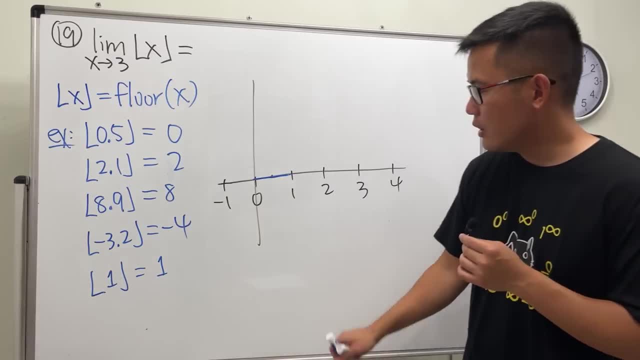 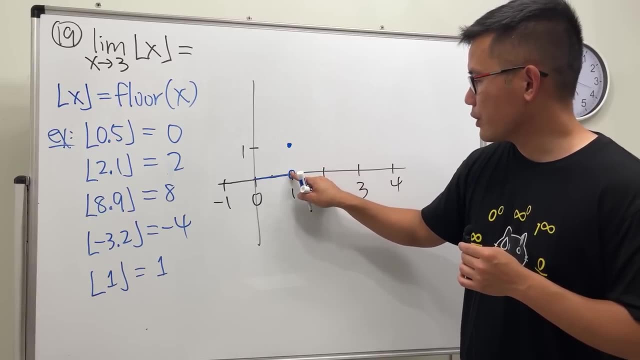 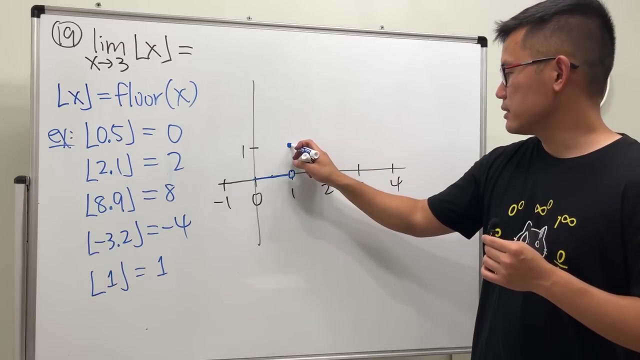 if this is a whole number already, then you just get that whole number back. so when x is 1, you jump to 1. so you have a closed circle here and you have an open circle here, and then you continue. when we have 1.1, flow of that is 1, likewise anything up to almost. 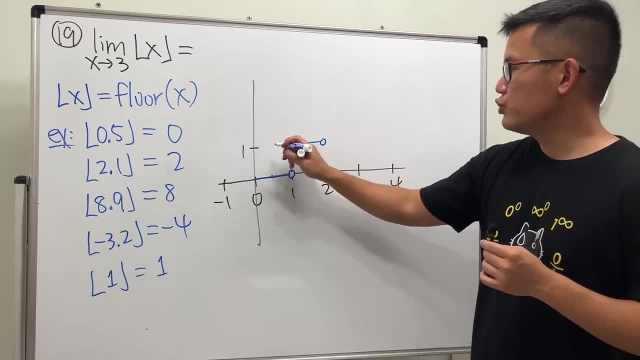 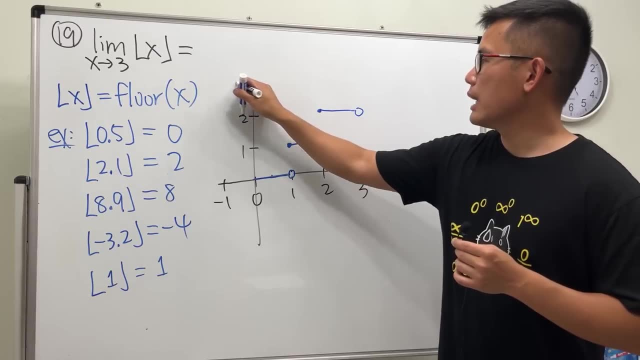 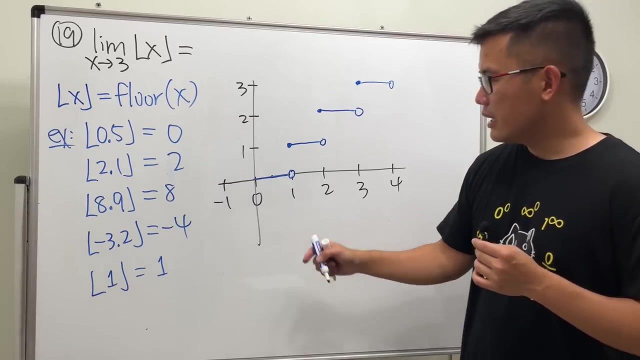 2, because when x is exactly 2, we make another jump to 2, same thing open, and then up 3, and then here and then like this, and then so on, so on, so on, and, if you would like, when x is 0 you get 0, and then 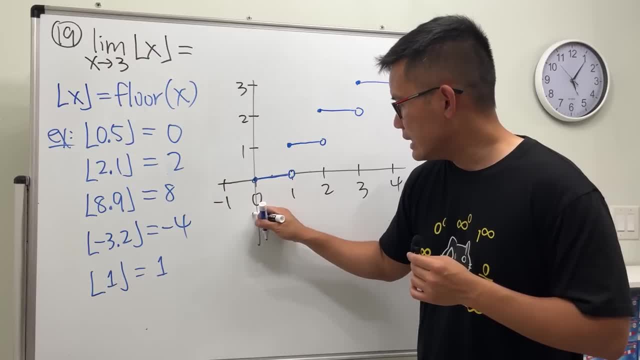 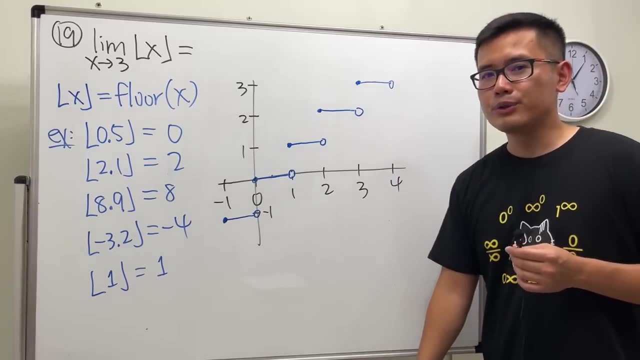 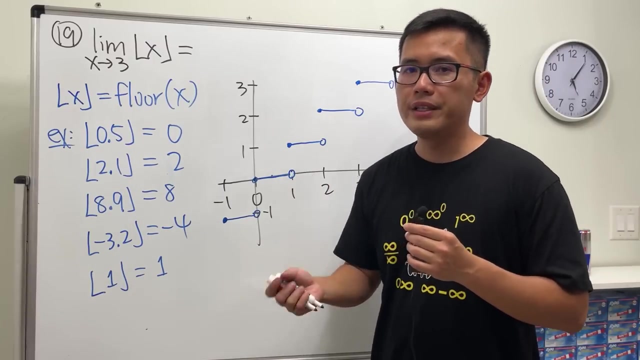 anything from negative 1 to here we get negative 1, so you have a piece like this. so it's like a stair. i believe some people also call this the stair function, but, like the flow function is the most common one or maybe the greatest integer function. but anyway, though, check this out when x. 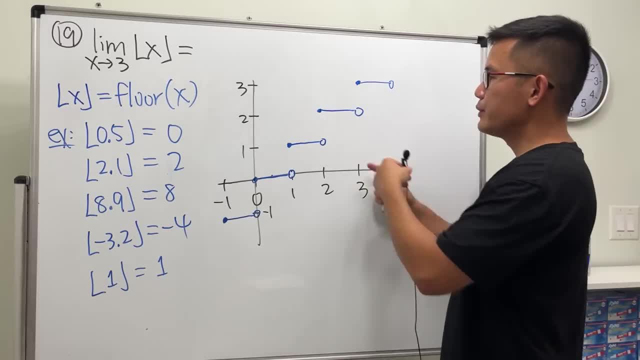 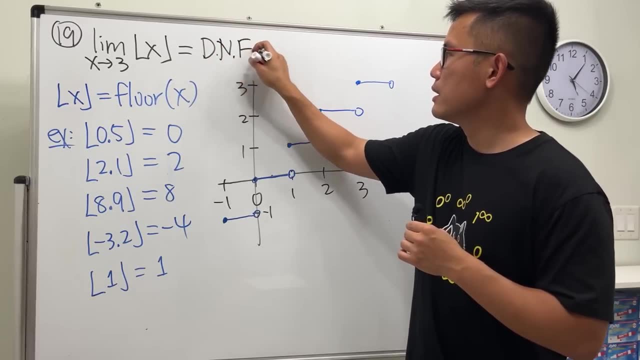 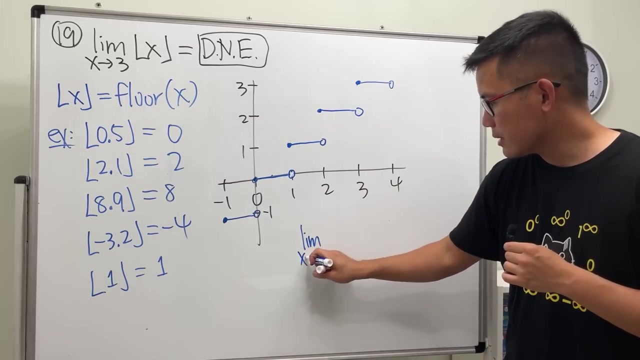 is approaching 3 from the left, we get 2. from the right, we get 3. so the answer for this right here doesn't exist. and let me just indicate that real quick. if we have the limit as x approaching 2- sorry, if we have the limit as x approaching 3 from the left hand side, so 3 minus of the flow function. 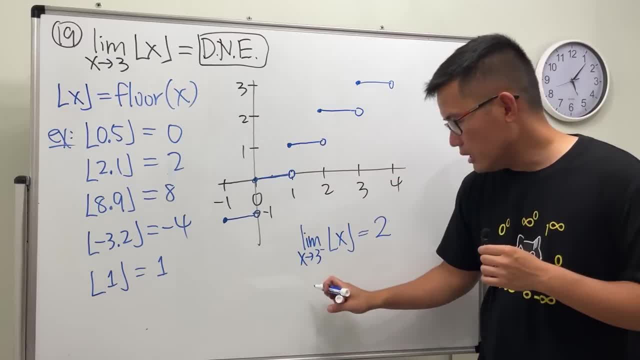 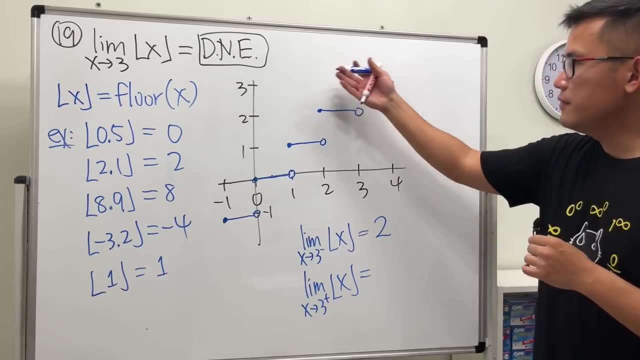 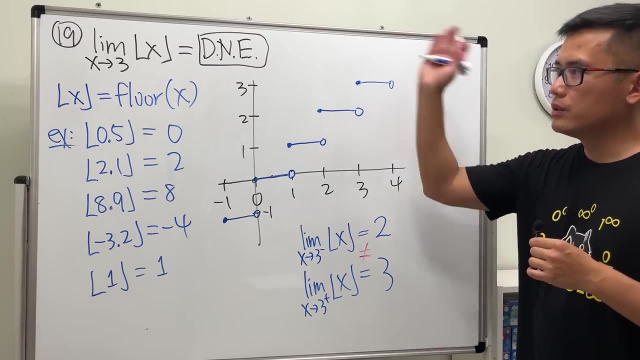 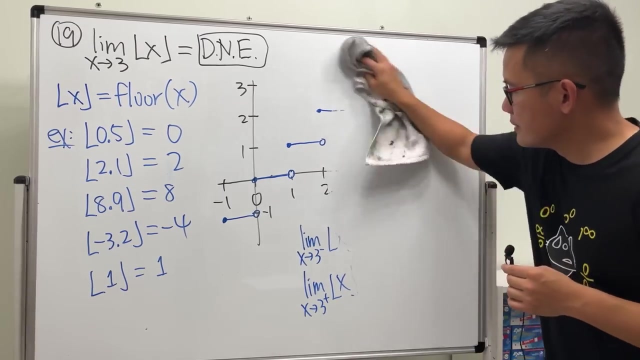 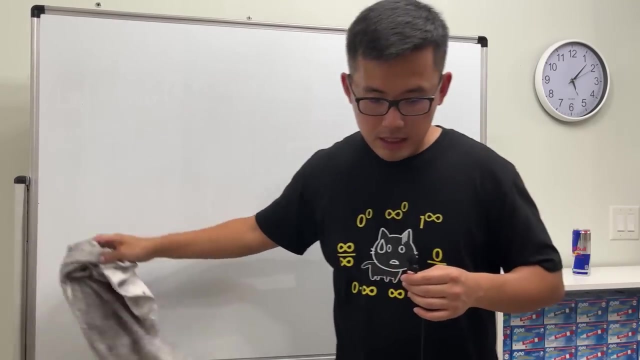 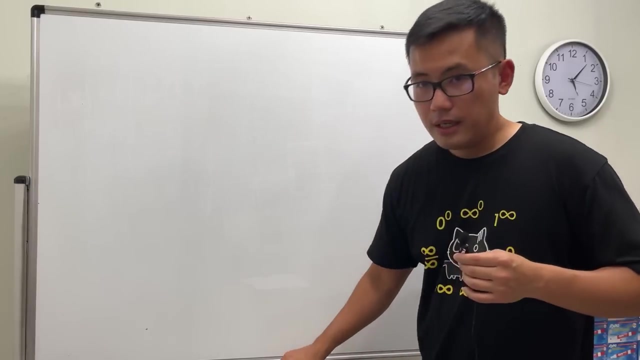 this right here gives us 2.. but if we have the limit as x approaching 3 positive, then this right here gives us 3.. unfortunately they are not equal, so we do not have the limit for it. okay, and depending on your calculus class, some people cover the special function that was one of the 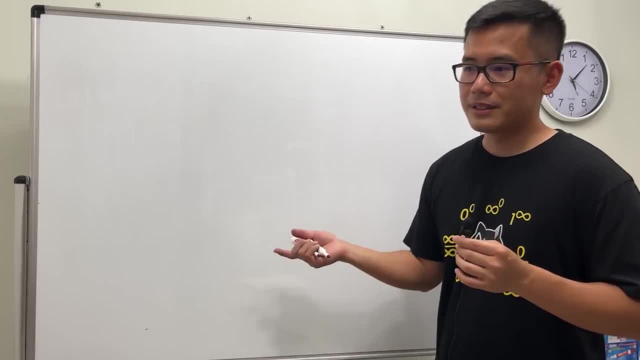 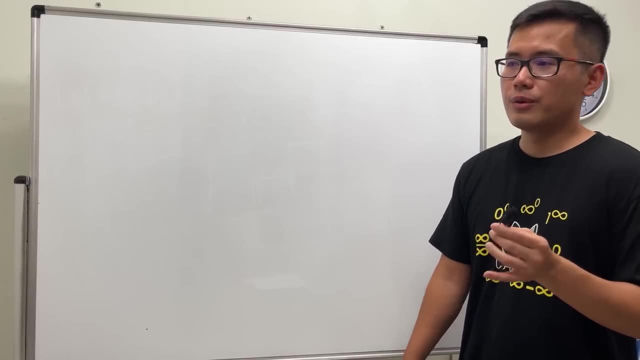 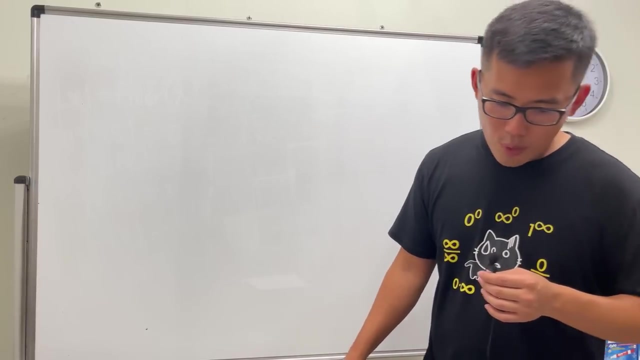 special functions, the flow function, um, most of the people we do, and we also cover the fractional part of the function. but like, yeah, anyway, number 20, yay here, limit as x to the right, so this is the limit as x to the left. so this is the limit as x to the right. 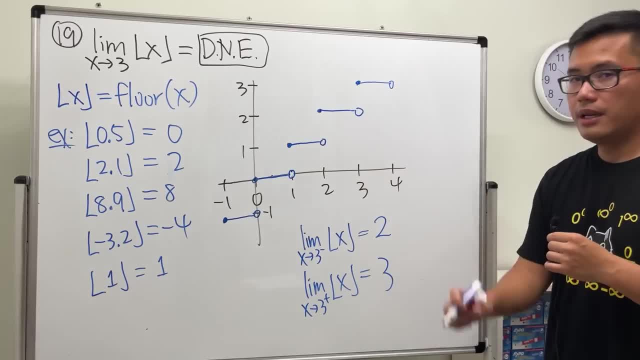 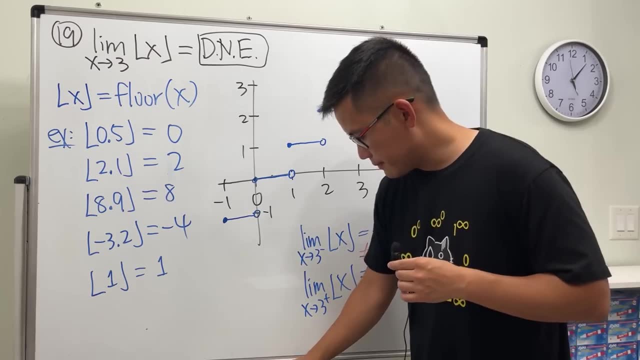 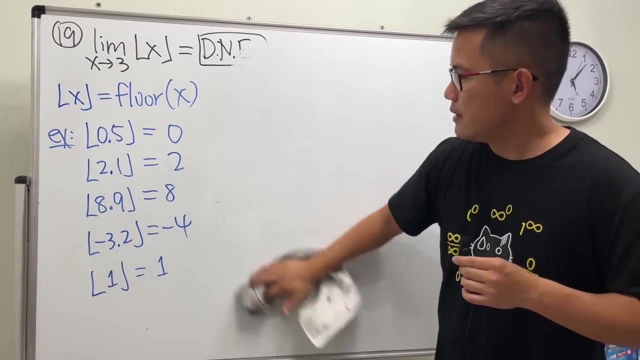 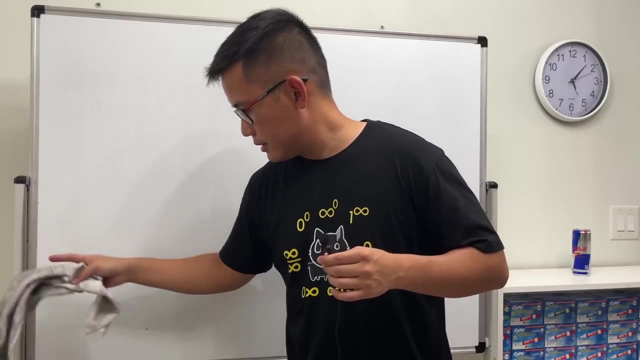 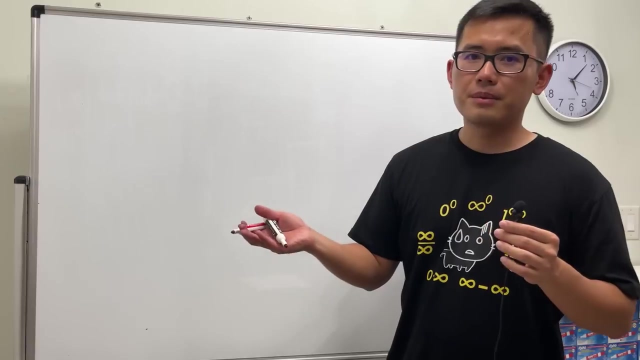 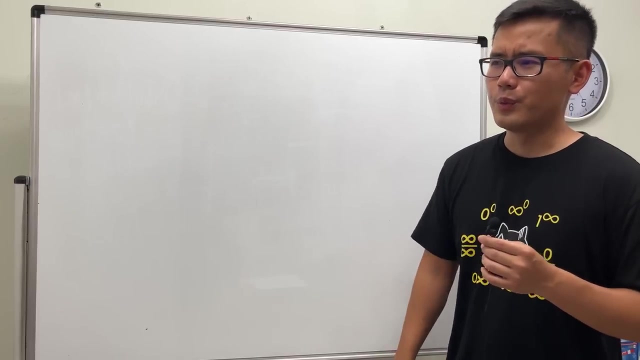 then this right here gives us three. unfortunately they are not equal, so we do not have the limit for it. okay, and depending on your calculus class, some people cover the special function- that was one of the special functions- the flow function. most of the people we do, and we also cover the fractional. 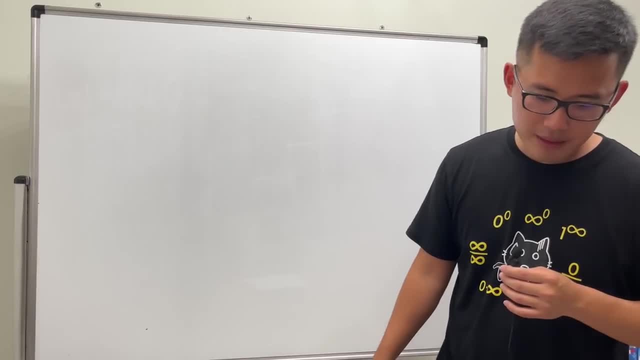 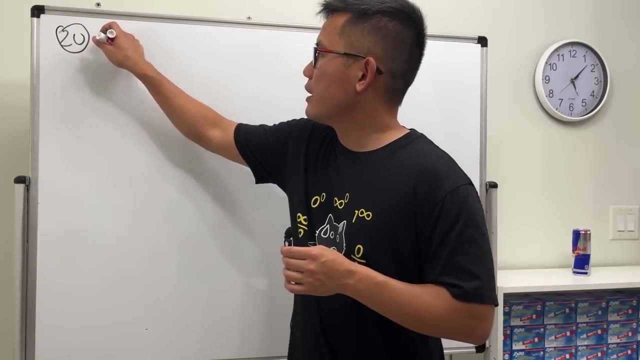 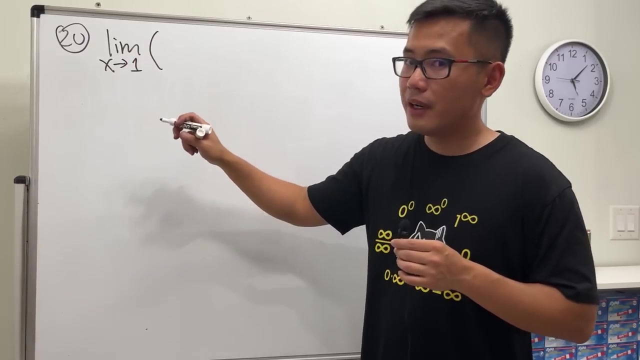 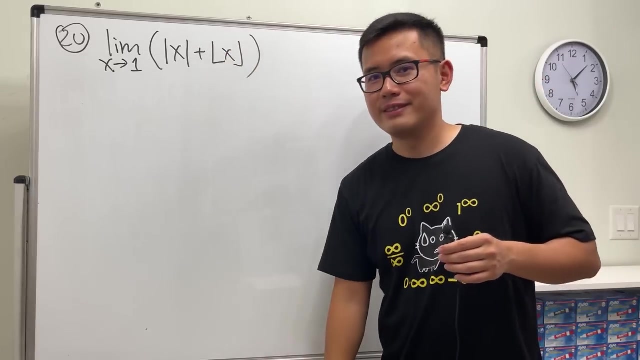 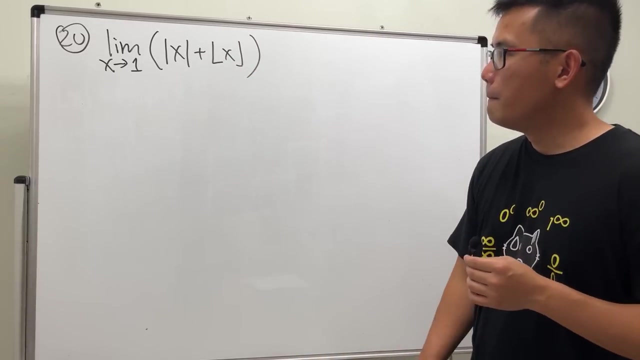 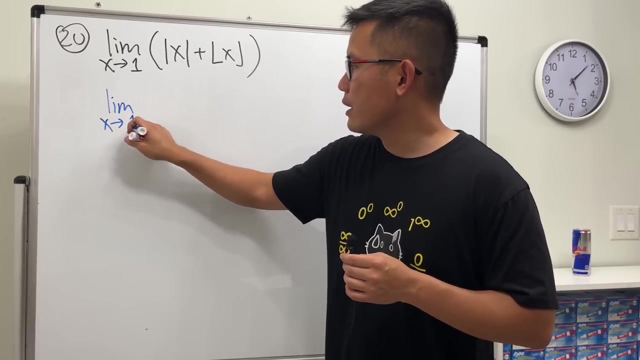 part of the function. but like, yeah, anyway, number 20, yay, here, limit as x approaching one, and the function here is absolute value of x plus the flow of x. wow, okay, let me just show you guys how we can do this. um, yeah, now let's just do without the graphs if x is approaching one. 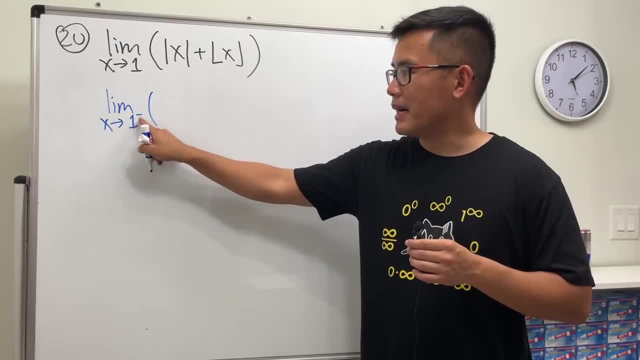 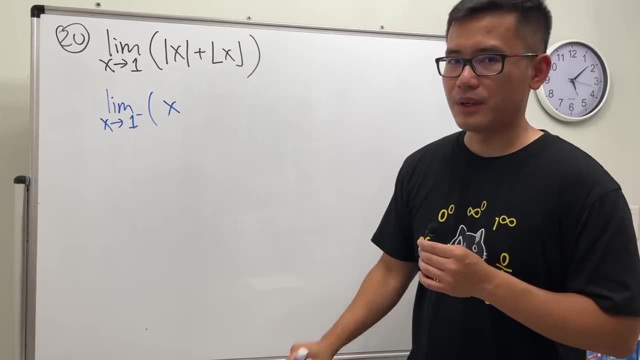 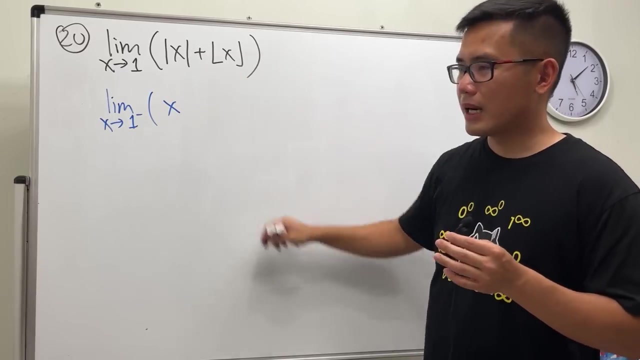 from the negative direction. guess what? because it's one minus. so this right here is still just x, right? so we just have x. just take out the opposite, for it doesn't matter. and then, hmm, it's not so easy to write it, so perhaps i'll just. 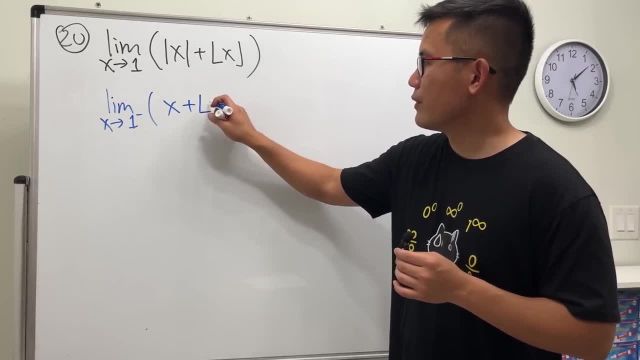 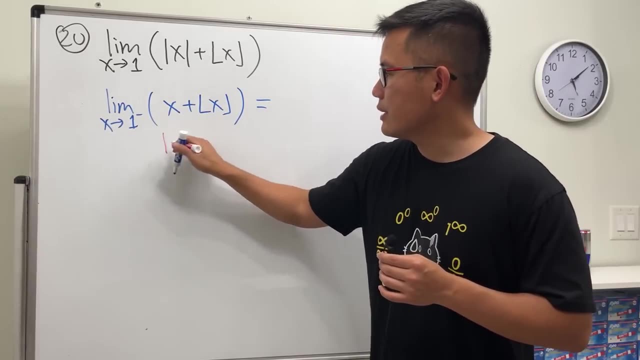 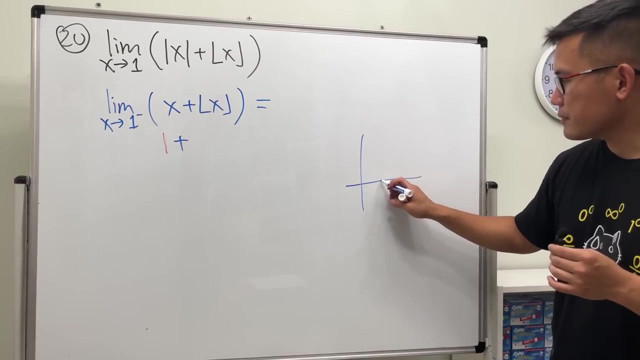 i, i think i'm just going to write it like this: plus the flow of x. yeah, and here's the deal: one minus is just like one right one and then plus. if you have one minus, what's the flow of one minus? well, if you look at the picture earlier, it's like this right, zero to. 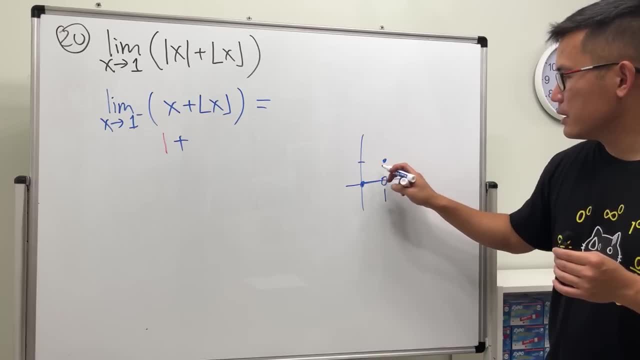 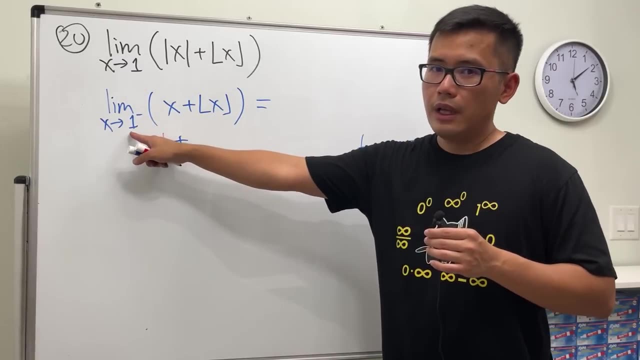 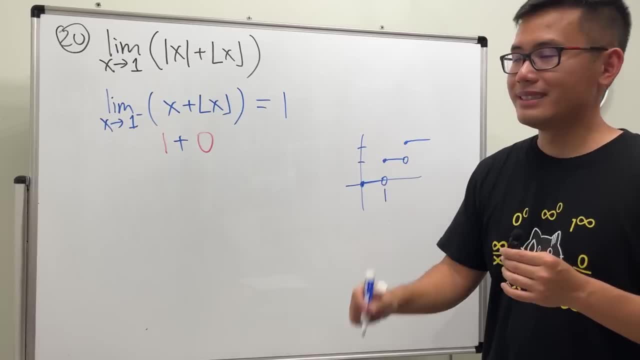 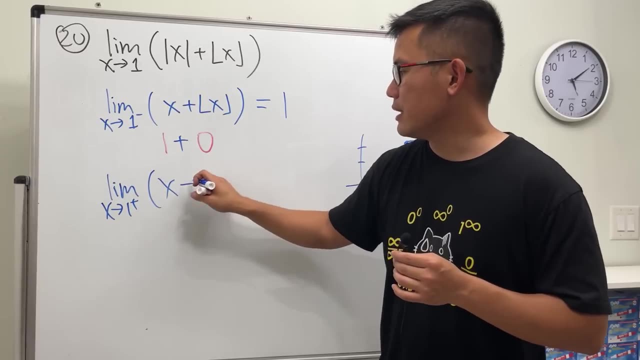 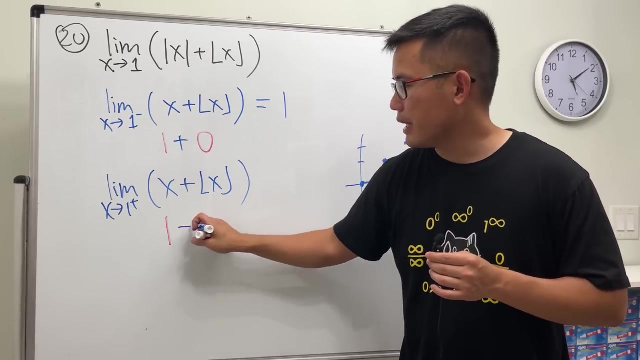 so it's one plus 0. so the answer for this one is one. but if we have the limit as x approaching 1 plus, just take off the absolute value, doesn't matter. okay, that is going to be still one plus one plus. when we put it here it justsaw down right, so it's just one. so it's one plus 1. 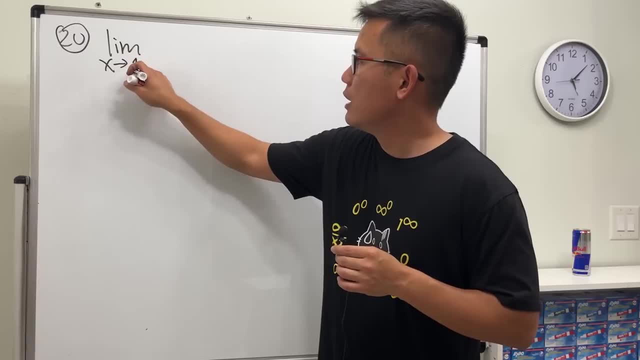 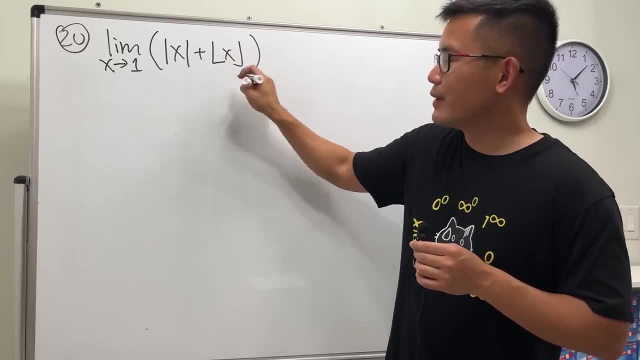 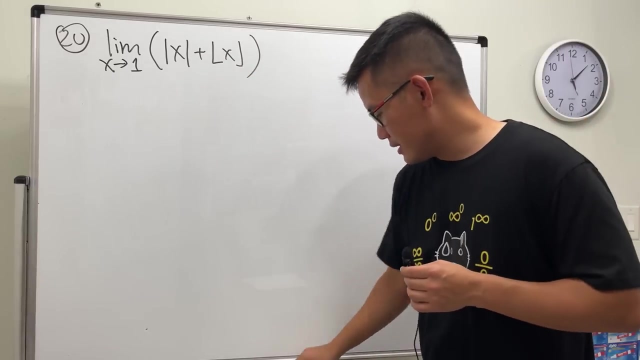 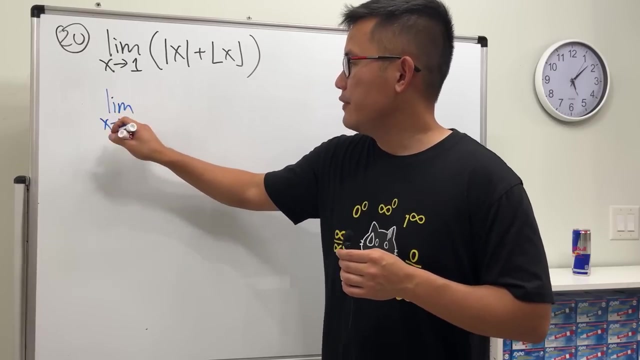 so we're going to have the limit as x to the left. so if x is approaching 1 and the function here is absolute value of x plus the flow of x, wow, okay, let me just show you guys how we can do this. yeah, now let's just do without the graphs if x is approaching one from the negative direction, guess what? because it's one minus. 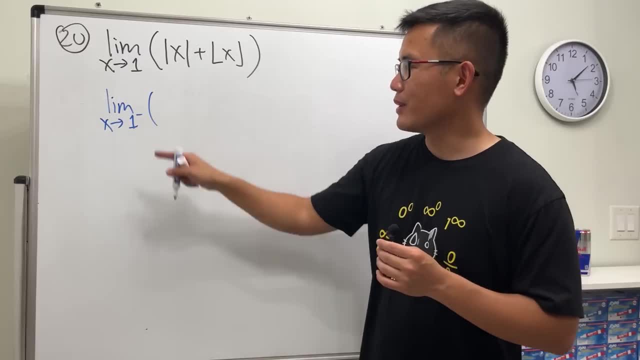 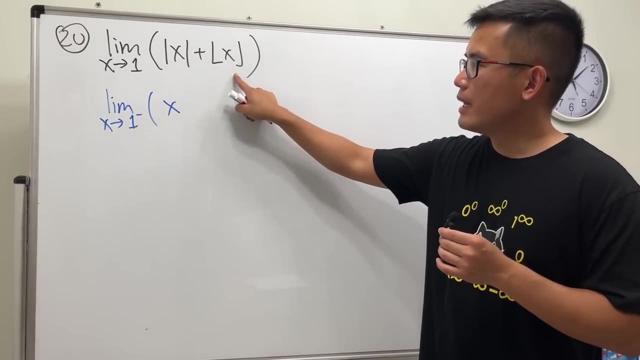 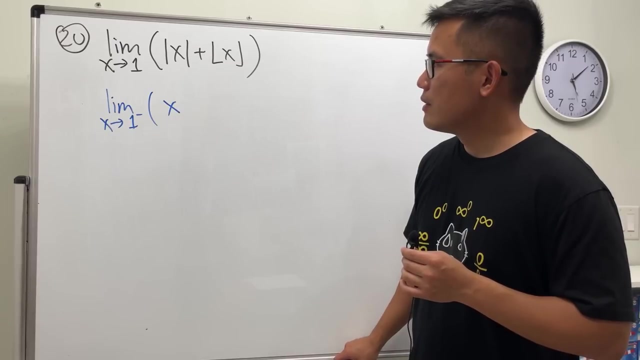 so this right here is still just x, right, so we just have x. just take out the opposite part, doesn't matter. and then, hmm, it's not so easy to write it, so perhaps i'll just- i, i think i'm just going to write it like this, plus the full of x. 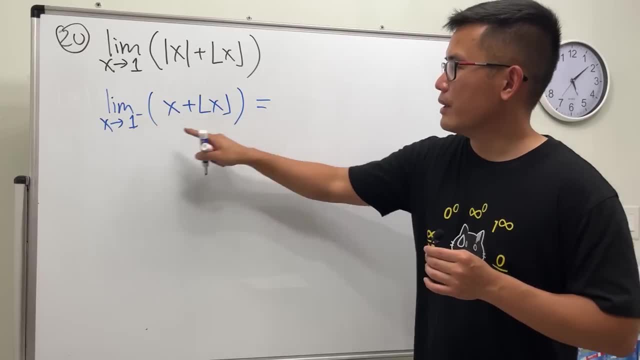 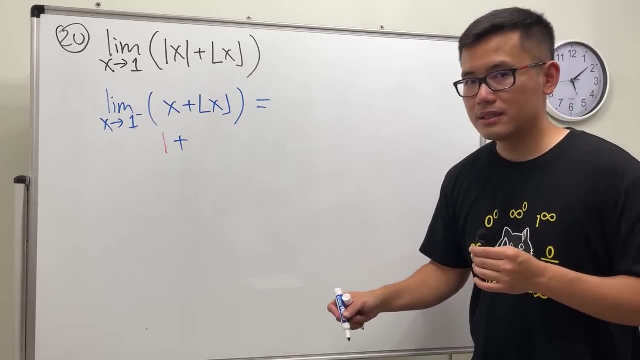 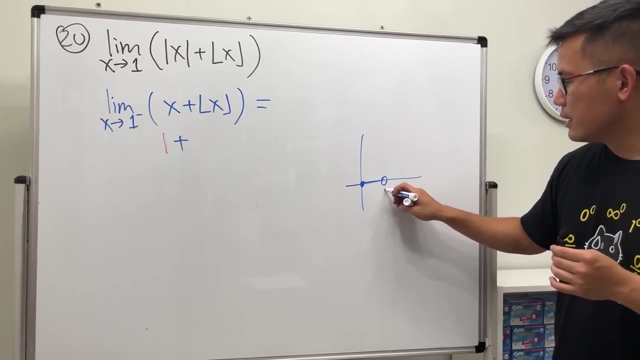 yeah, and here's the deal: one minus is just like one, right one and then plus. if you have one minus, what's the full of one minus? well, if you look at the picture earlier, it's like this right zero to one, and then there's a jump and then like this, and then so on. 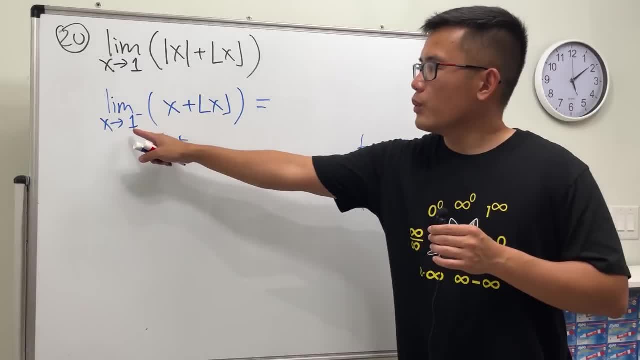 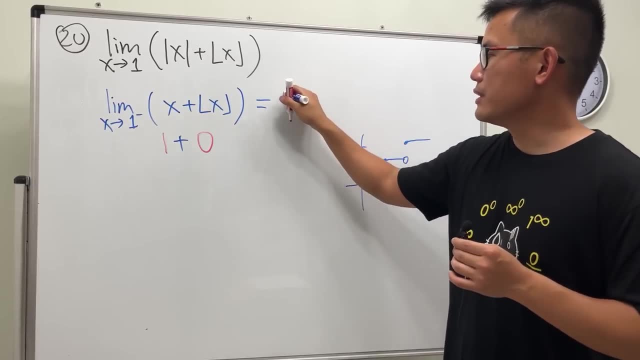 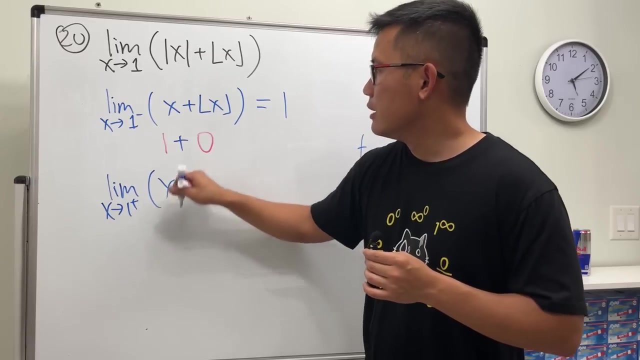 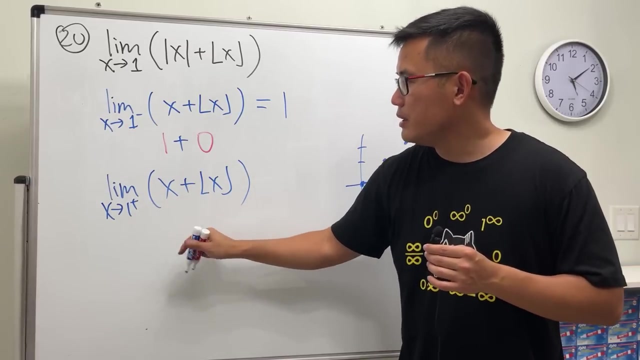 so when we have x is approaching one from the left hand side, it's zero. so it's one plus zero. so the answer for this one is one. but if we have the limit as x approaching one plus, just take out the absolute value. doesn't matter. okay, that is going to be still one plus, one plus. when we put it here, it just. 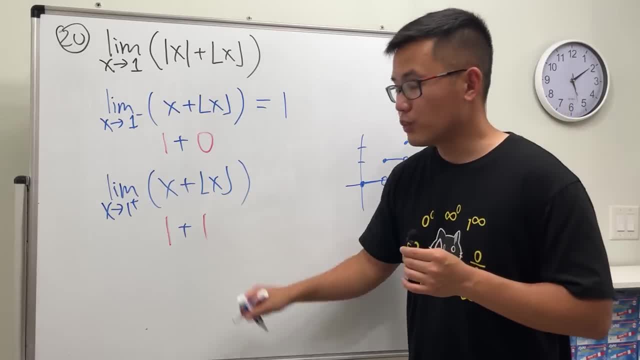 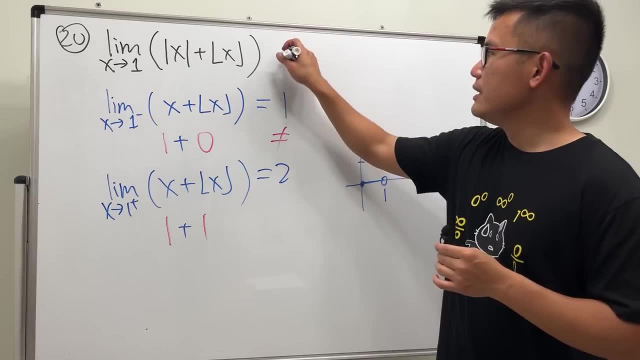 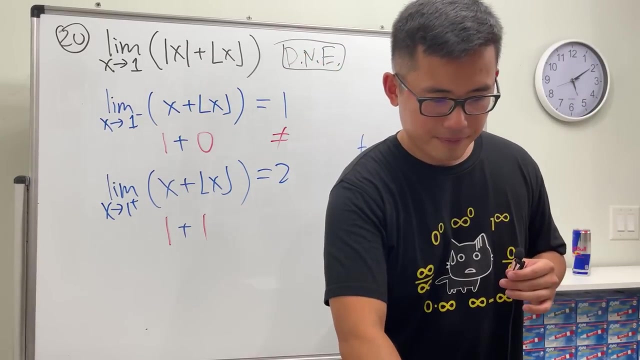 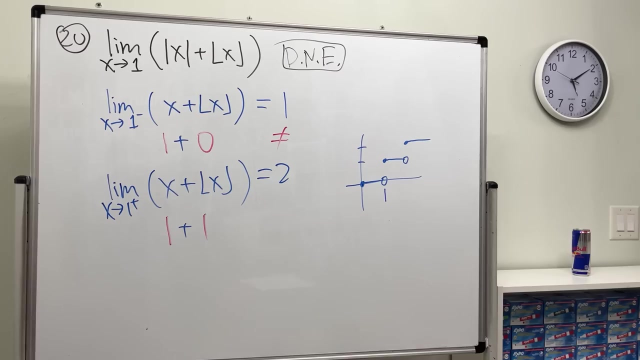 run down right, so it's just one. so it's one plus one, two, yes, but they are not equal, therefore. therefore, the answer for this, right here, dne, right, so yay. 20 questions done, and now let's have a look. one hour and 34 minutes. 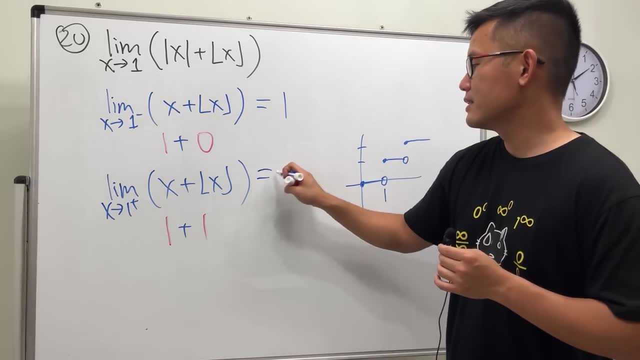 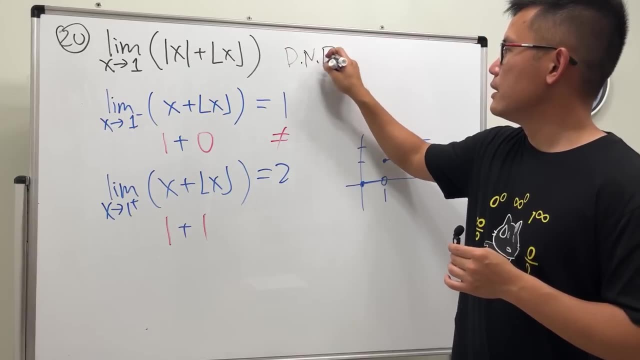 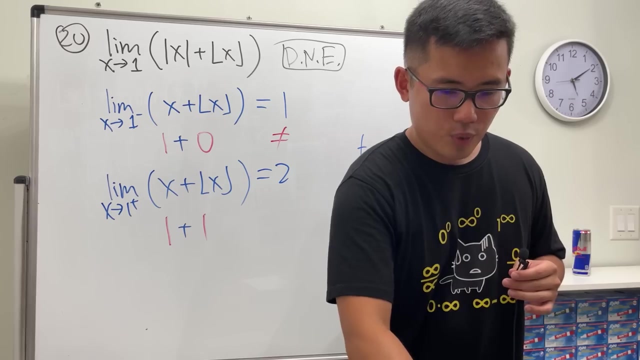 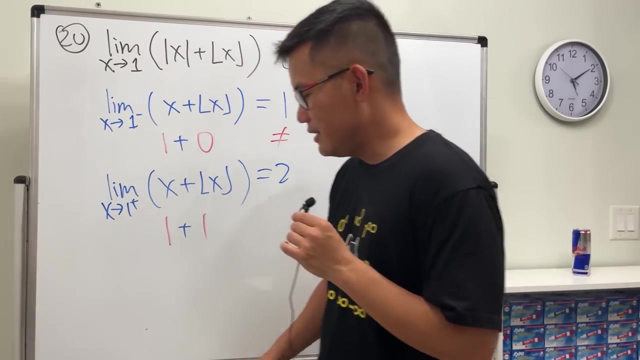 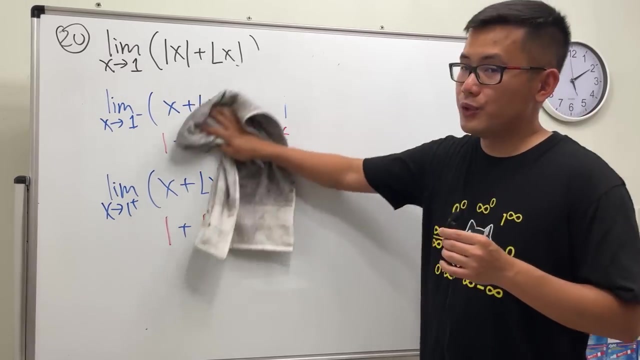 okay, so one plus one. so one plus one, one two, yes, but they are not equal. therefore the answer for this right here: d and e, all right, so yay, 20 questions done. and now let's have a look. one hour and 34 minutes, okay, so on page four, we are going to just compute the limit, so no more graphs. 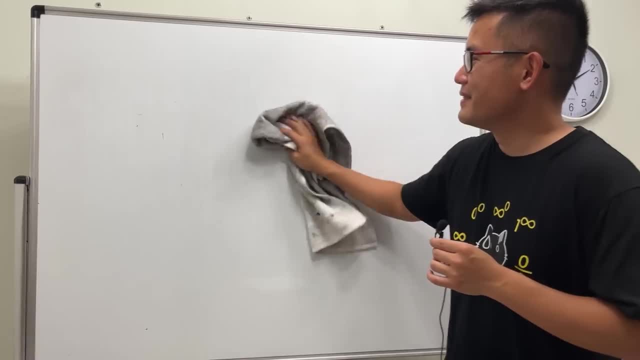 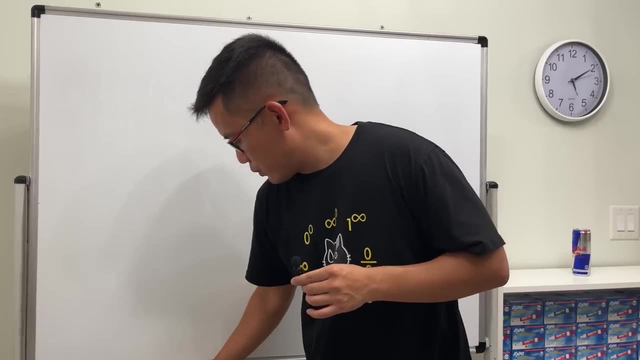 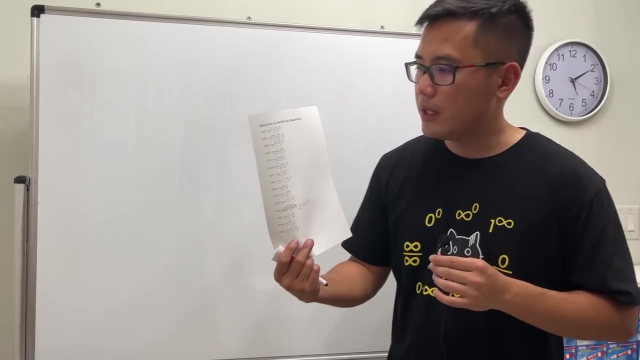 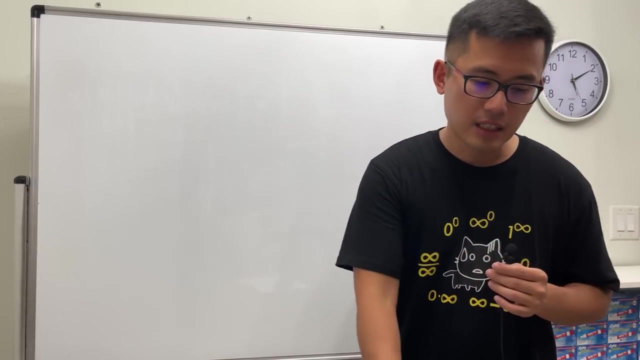 so that's good, because the graph took a while to do, right, all right. and also we are just going to be doing algebra. so this is going to be the limit as x approaching some number a, and for now a is finite in this category. and i'll show you guys the techniques, the things. 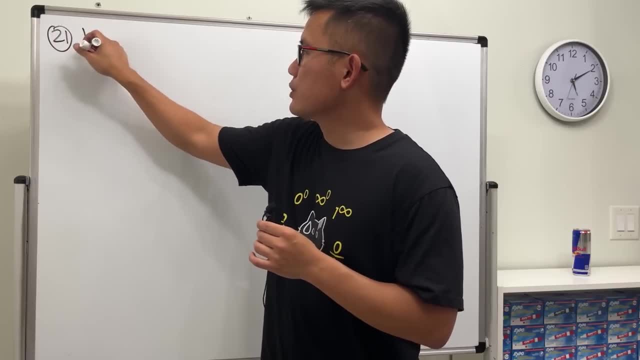 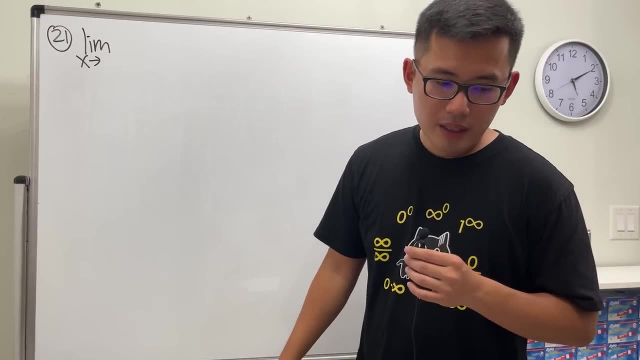 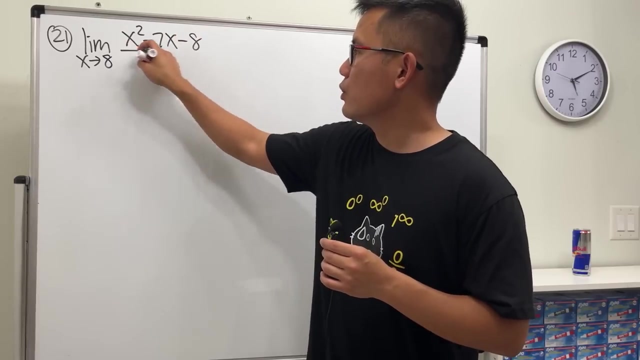 that we will have to do to figure out the limits, and i'll also show you guys how to organize our work and all that good stuff. first question on page number four, number 21, the limit as x approaching eight, x square minus seven, x minus eight over x minus eight. first thing first. 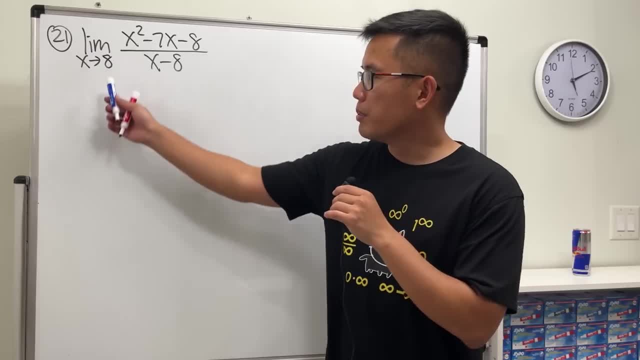 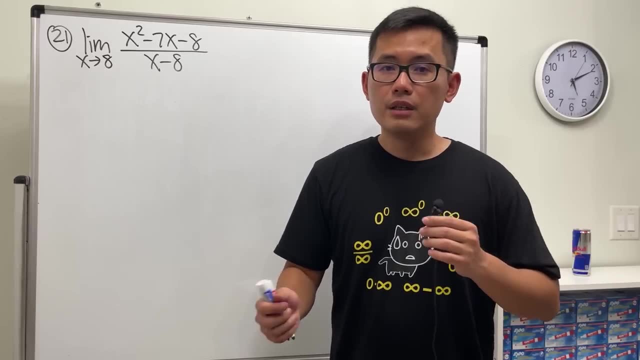 when we are just computing the limit, it's always a good habit to plug in this number into all the x's and see what happens. if we get a nice number, then that will be our nice answer. if we end up with one of these numbers, well, i should have said one of these- limit indeterminate. 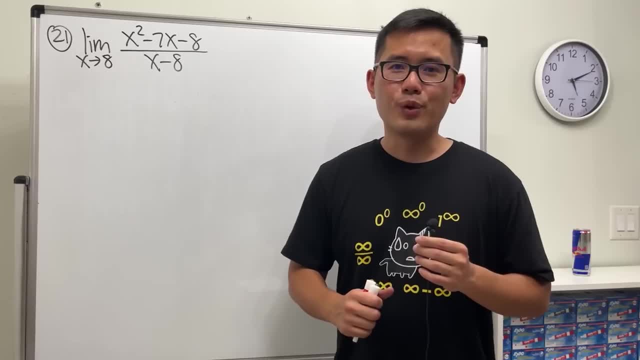 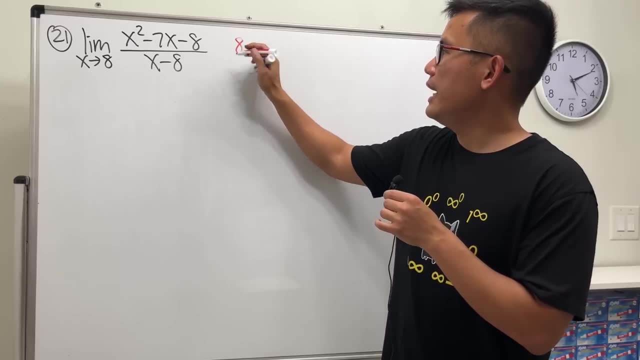 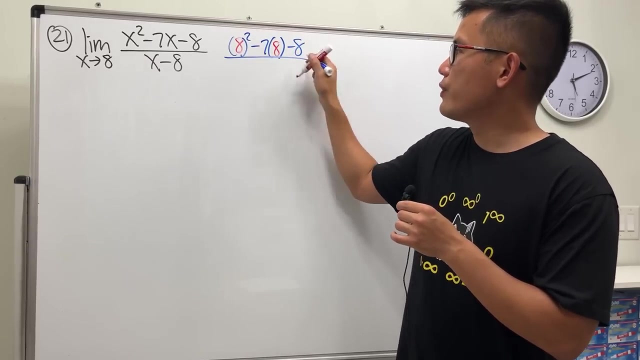 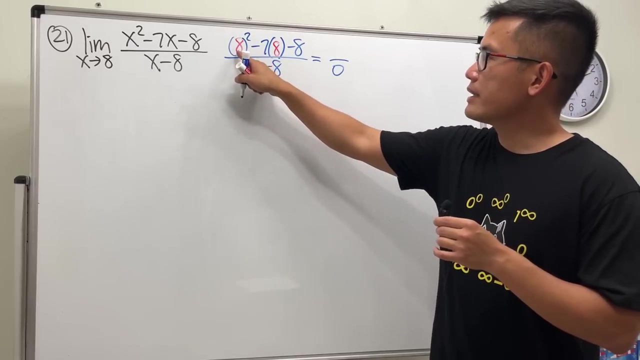 forms, then congratulations. we will have to do more work. so let's see, i will show you guys all the work for now. put the eight into all the x's, then we are going to get eight square minus seven times eight, and then minus eight or over eight minus eight on the bottom, we get zero on the top. this is 64. 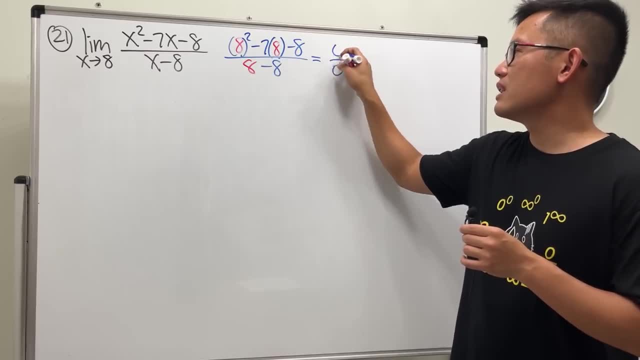 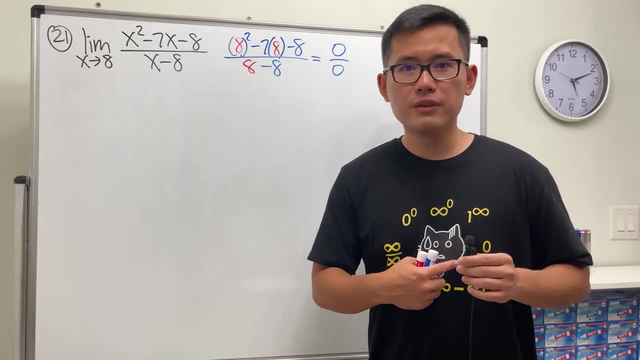 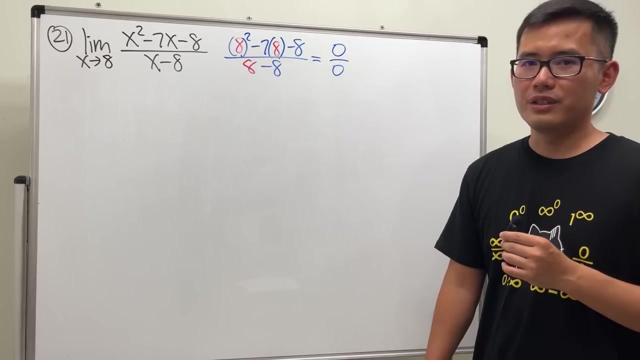 minus 56, which is 8, and then minus 8, which is 0, 0 over 0. we cannot draw any conclusion why? because is one of the indeterminate forms. the cat is scared. we are scared of indeterminate forms. we cannot draw any conclusion yet, but don't worry, i'll show you how to take care of this. 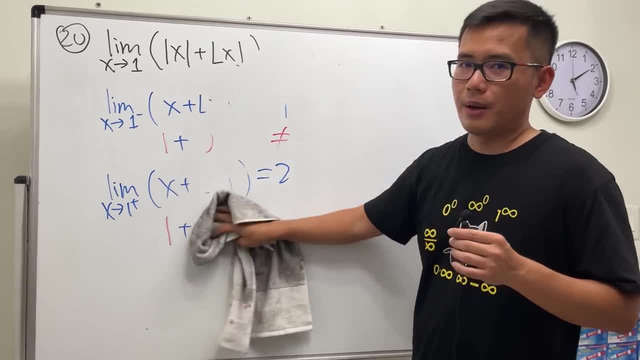 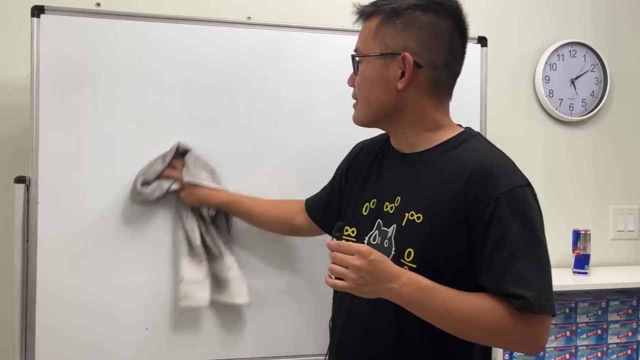 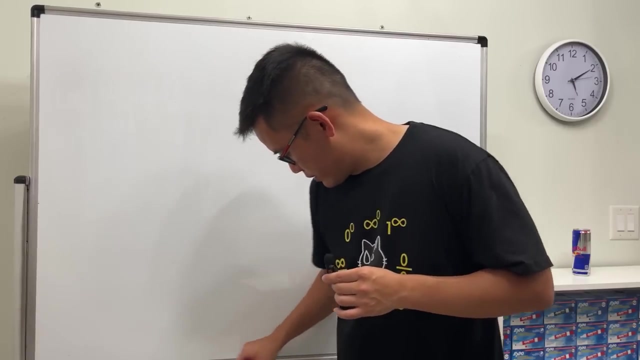 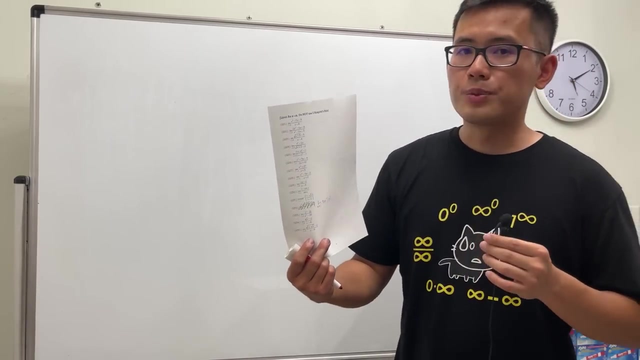 okay, so on page four we are going to just compute the limit. so no more graphs. so that's good. so thisness graph took a while to do, right, oh, all right. and also we are just going to be doing algebra, so this is going to be the limit. 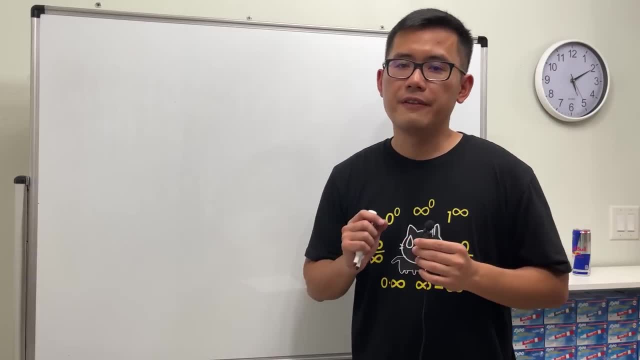 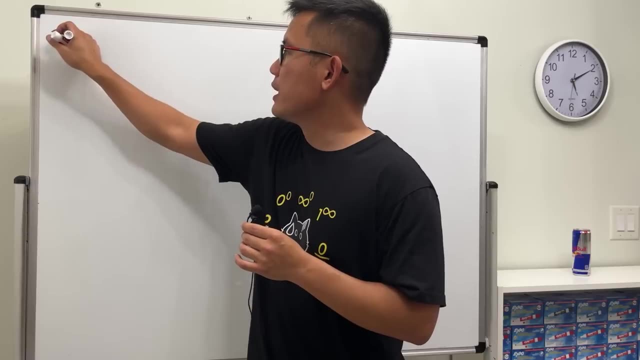 as x approaching some number a- and for now a is finite, uh, in this category, and i'll show you guys the techniques, the things that we will have to do to figure out the limit as x approaching some number a, and out the limits, and i'll also show you guys how to organize our work and all the good stuff. first, 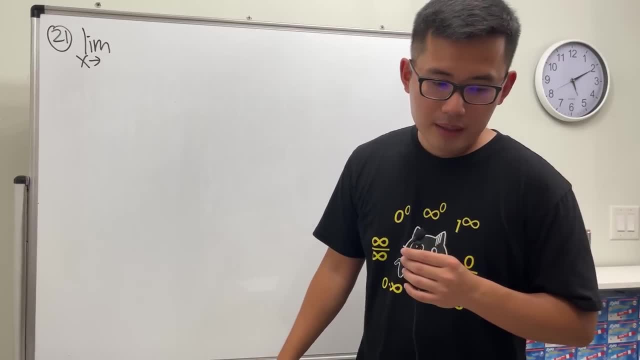 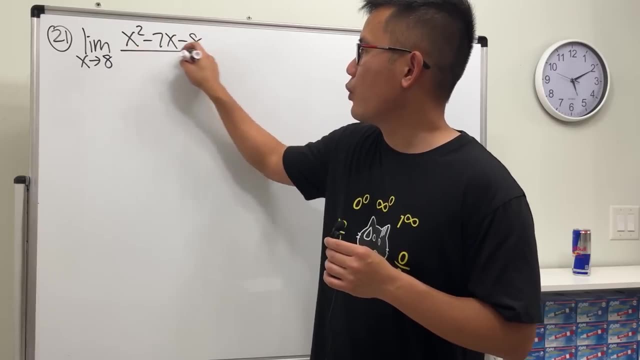 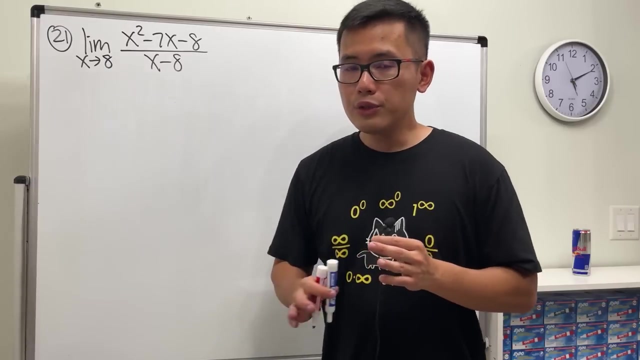 question on page number four, number 21, the limit as x approaching eight, x square minus 7x minus 8 over x minus 8.. first thing first. when we are just computing the limit, it's always a good habit to plug in this number into all the. 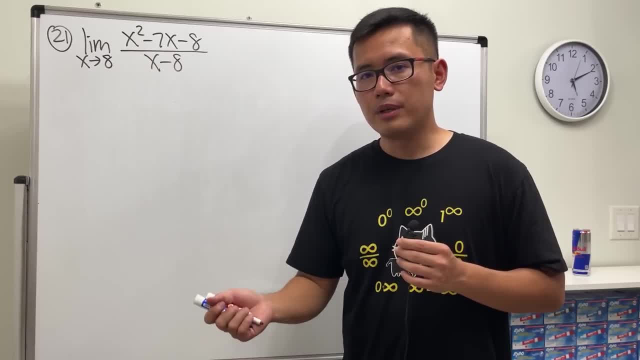 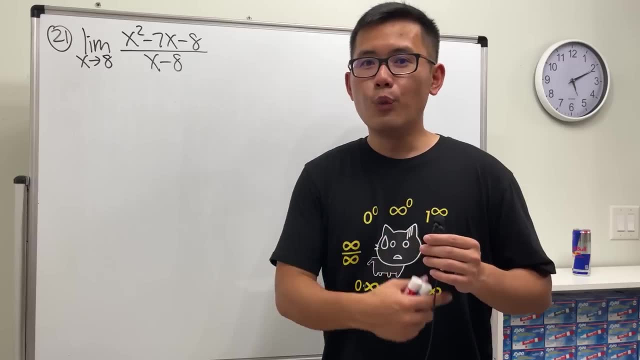 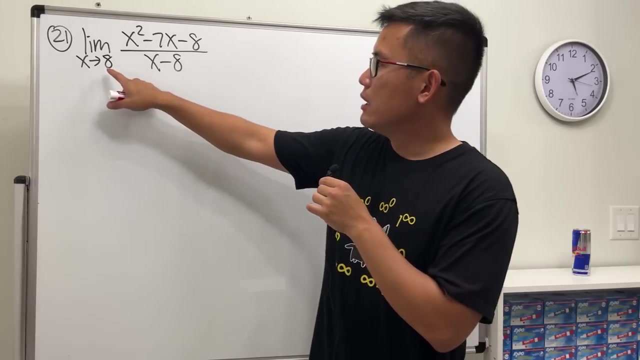 x's and see what happens. if we get a nice number, then that will be our nice answer. if we end up with one of these numbers- well, i should have said one of these limit indeterminate forms- then congratulations. we will have to do more work. so let's see, i will show you guys all the work for. 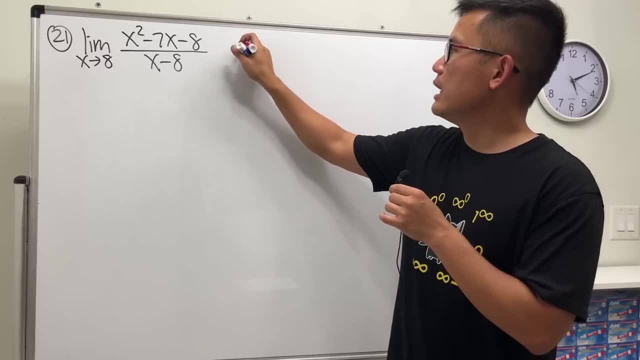 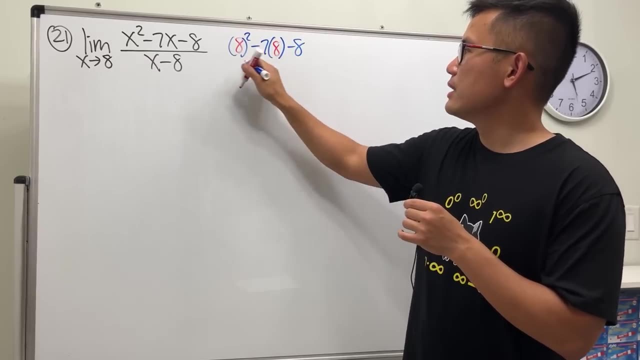 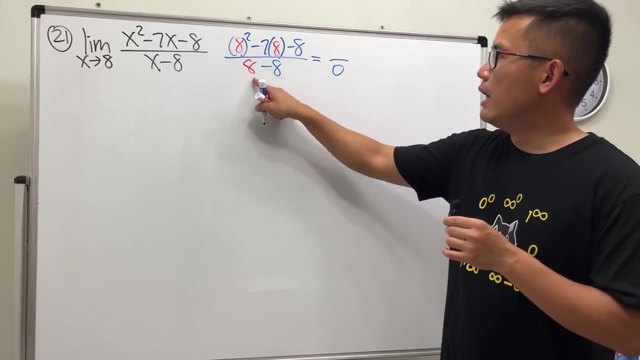 now put the 8 into all the x's, then we are going to get 8 square minus 7 times 8, and then minus 8, or over 8 minus 8. on the bottom, we get 0. on the top, this is 64 minus 56, which is 8, and then minus 8, which. 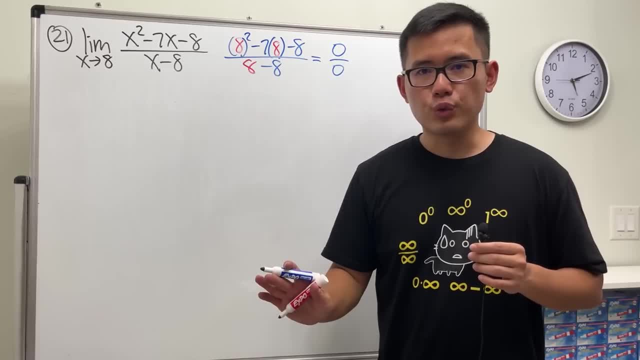 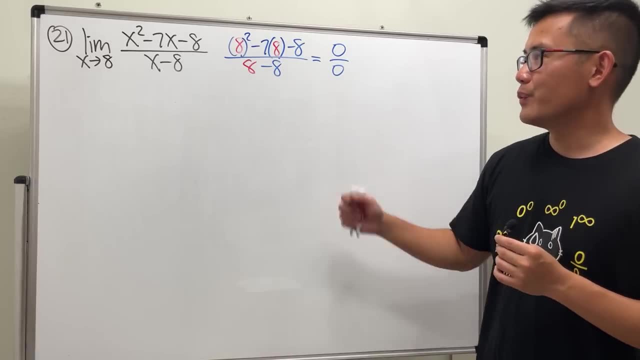 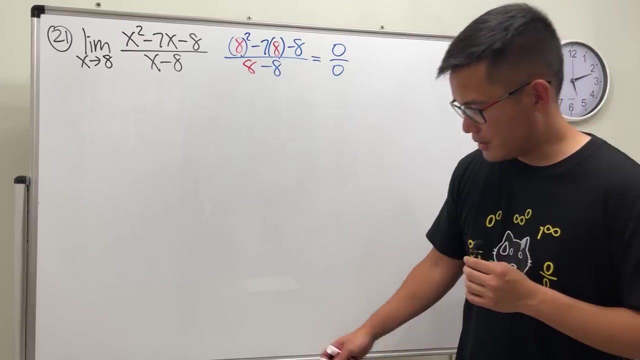 is 0, 0 over 0, we cannot draw any conclusion. why? because it's one of the indeterminate forms. the cat is scared. we are scared of indeterminate forms. we cannot draw any conclusion yet, but don't worry, i'll show you how to take care of this. 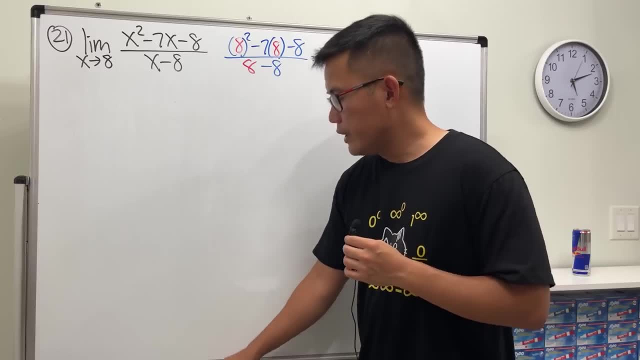 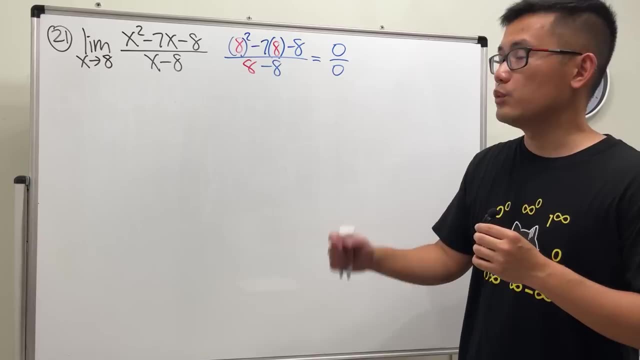 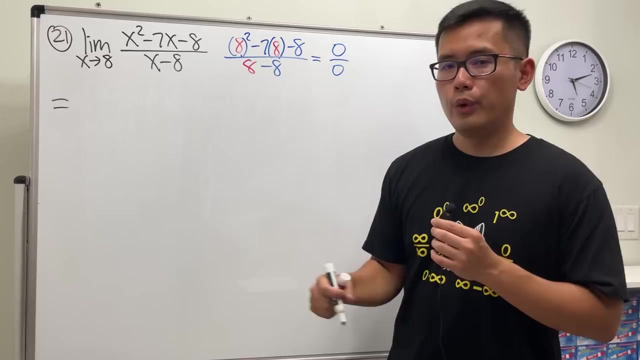 here's the deal: if we get 0 over 0- and we have that- then we can expect to cancel a common factor and in this case it will be the x minus 8.. to make that happen- notice the top is just a quadratic trinomial. we can actually just factor it the usual way. 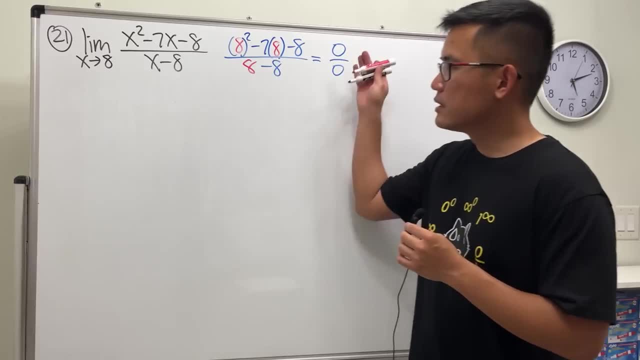 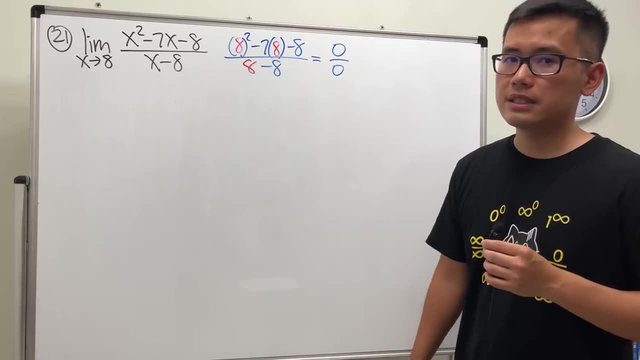 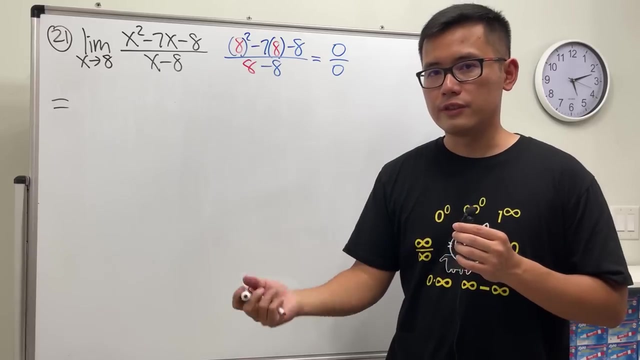 here's the deal: if we get zero over zero- and we have that- then we can expect to cancel a common factor, and in this case it will be the x minus eight to make that happen. notice: the top is just a quadratic trinomial. we can actually just factor it the usual way and then we will just get the. 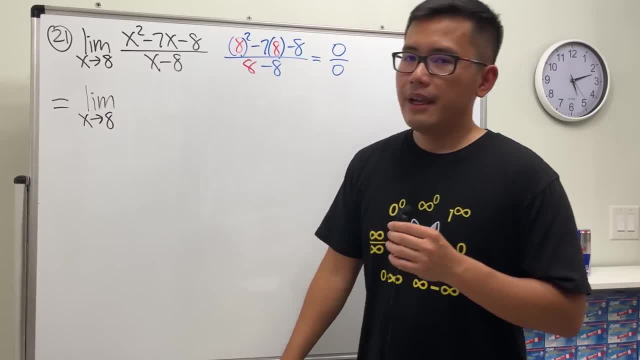 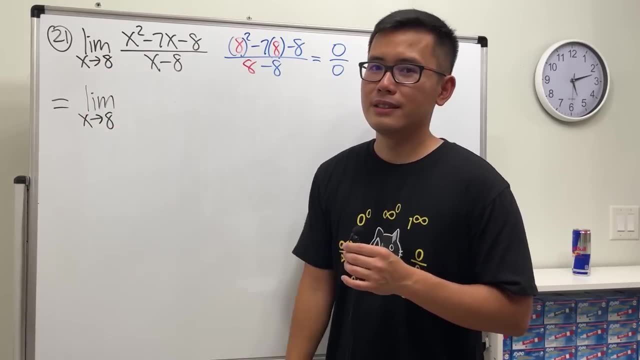 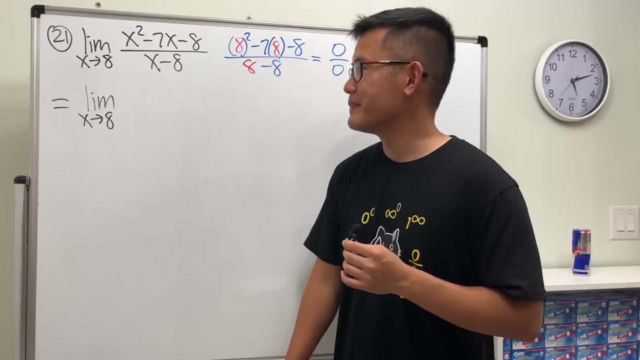 limit as x approaching eight and please, please, please, when you are doing this kind of limits, write down the lim x approaching eight. your teacher, your professor, will really appreciate that. i will also. yeah, later you'll see why that this is needed, especially once we get to the 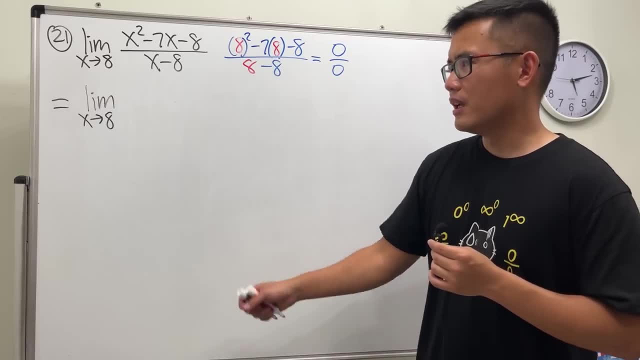 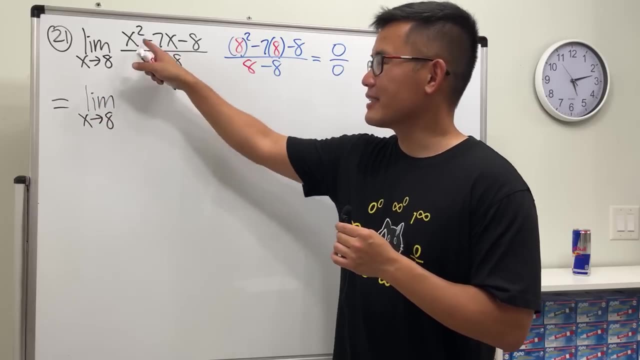 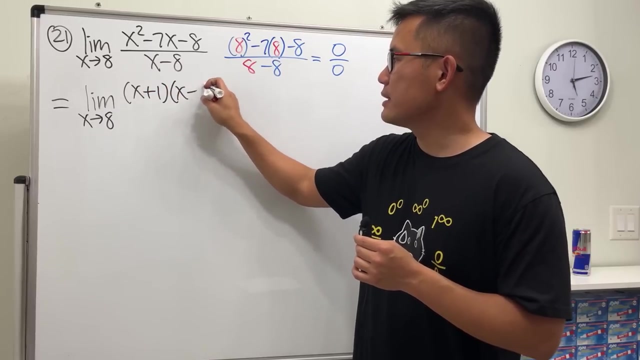 definition of derivative when there are a lot of variables being involved. so it's not, we are just being picky, it's actually necessary, all right. anyway, though, write this down and then, on the top, let's factor it. we will get x plus 1 times x minus 8, because this times out would be negative 8. 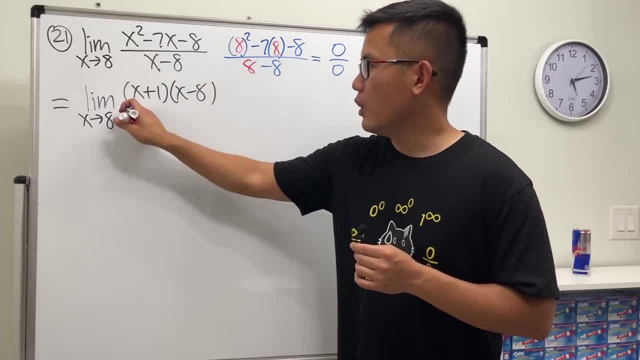 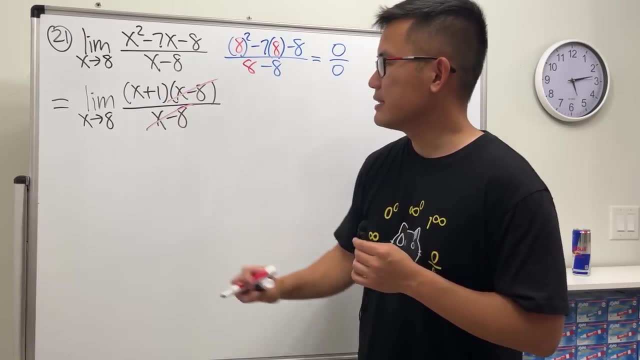 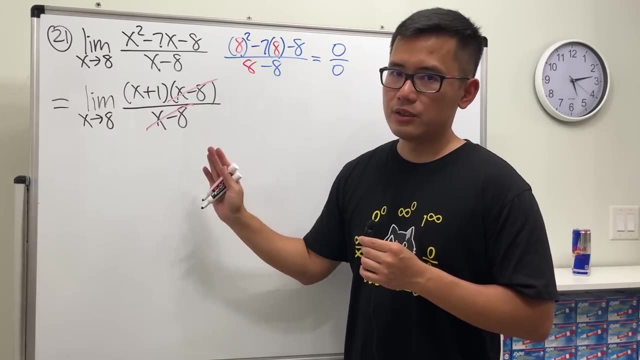 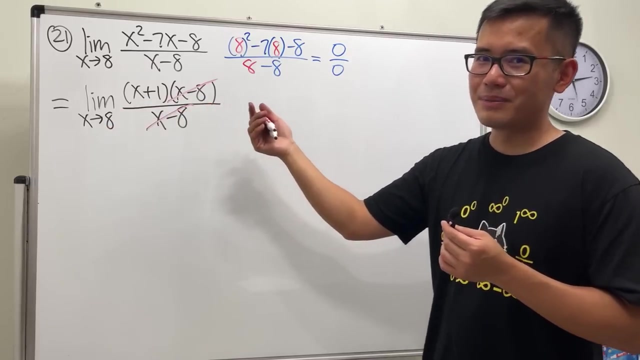 together we do produce the negative: 7x over x minus 8.. have a look: x minus 8, x minus 8. cancel out so nicely. and once you cancel out this common factor, then you wouldn't get a zero over zero anymore, because you can see when we put the eight in here, eight plus one next number. that's the nice answer. 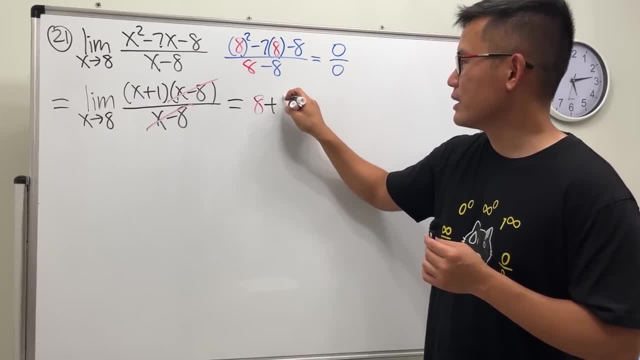 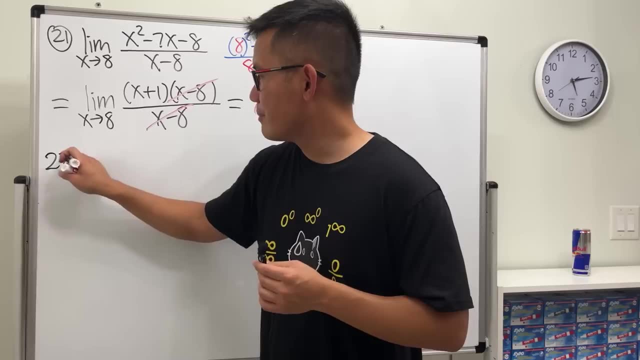 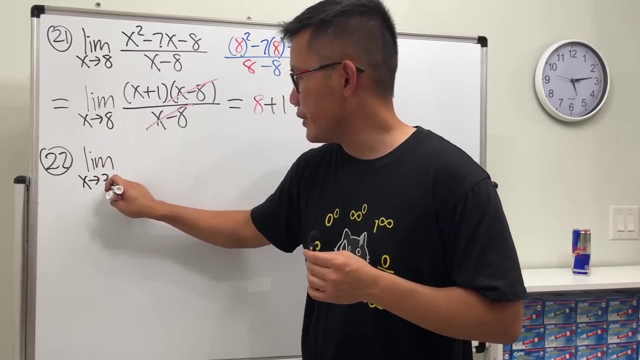 so now just go ahead. i'll show you guys the work. eight plus one, so the answer is nine, and then we are done. okay, so that's the answer for that. all right, number 22.. let's see, the limit is okay. so the limit is: x approaches three, and then we have. 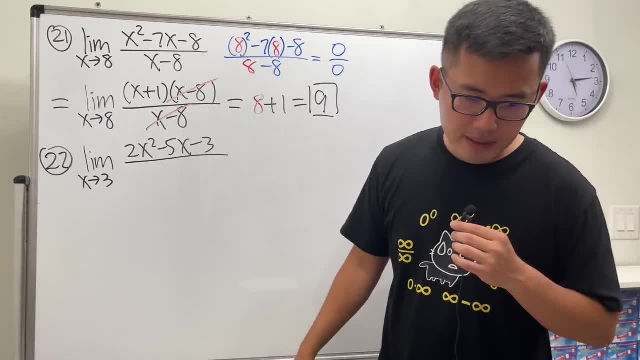 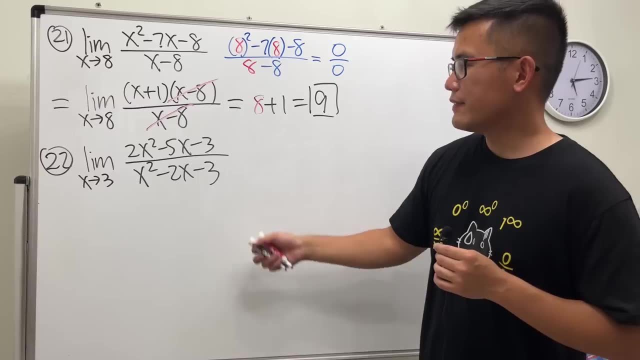 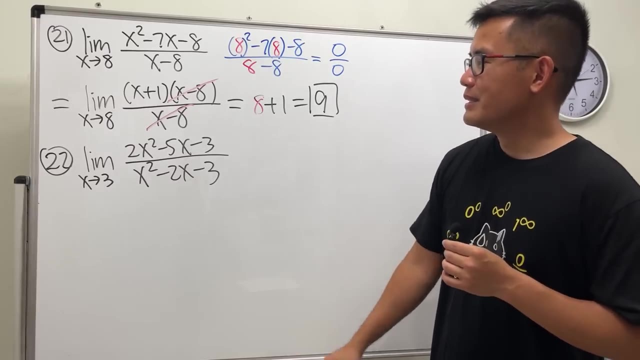 2x squared minus 5x minus 3, and on the bottom we have x squared minus 2x minus 3.. all right, so again, you should have a good habit not plugging the string to all the axes. you can work this out on your own. for, let's see, 3 in here is 9 times, that is 18. 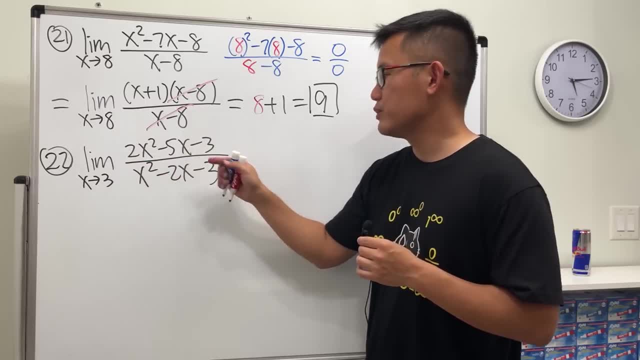 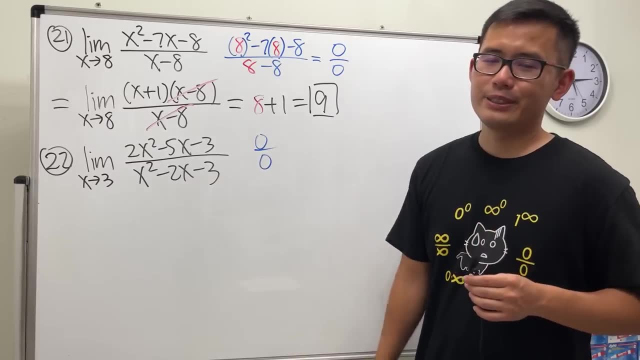 that's 15.. so 18 minus 15 is 3, 3 minus 3, we get 0. 9 minus 6 is 3 minus 3 is 0. so yeah, 0 over 0. do more work for this trinomial. trinomial, we can factor it, I'll show you. 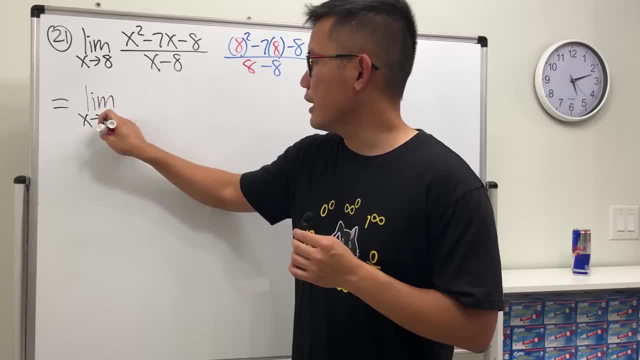 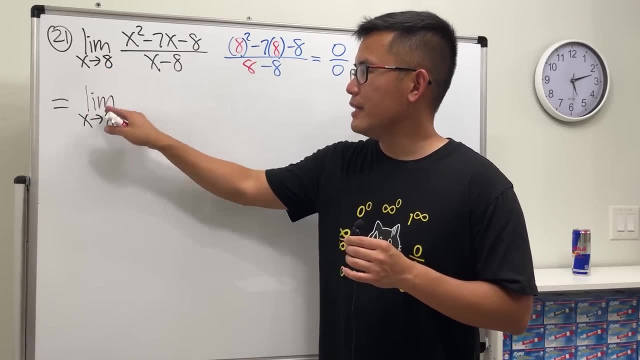 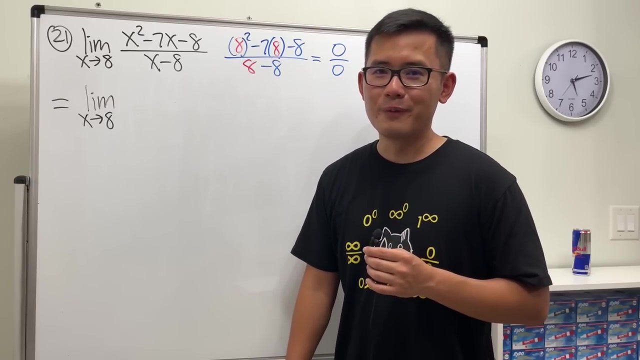 and then we will just get the limit as x approaching 8 and please, please, please, when you are doing this kind of limit, write down the l: i am x approaching 8.. your teacher, your professor, will really appreciate that. i will also. yeah, later you'll see why that this is needed, especially once we get to the definition of 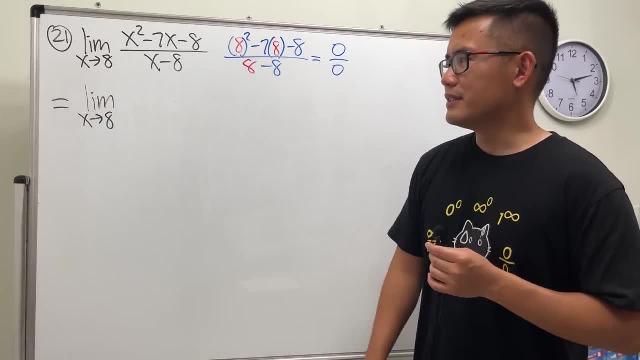 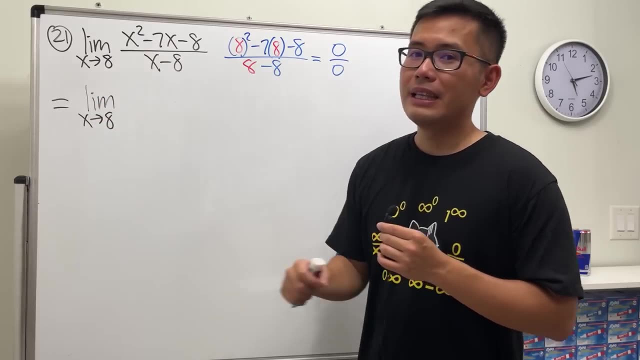 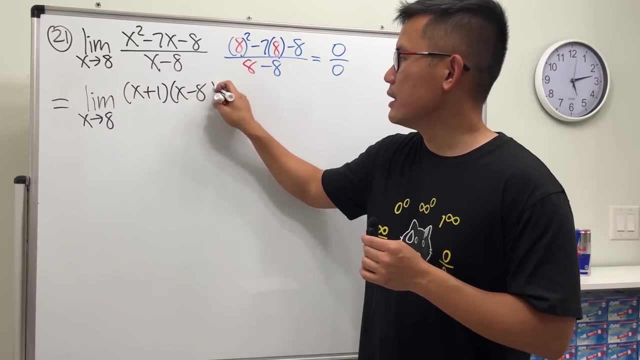 derivative when there are a lot of variables being involved. so it's not, we are just being picky, it's actually necessary. all right. anyway, though, write this down and then, on the top, let's factor it, we will get x plus 1.. times x minus 8, because this times out would be negative 8. together, we do produce the negative 7x. 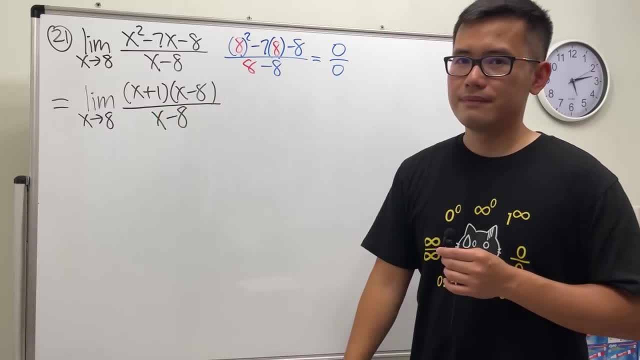 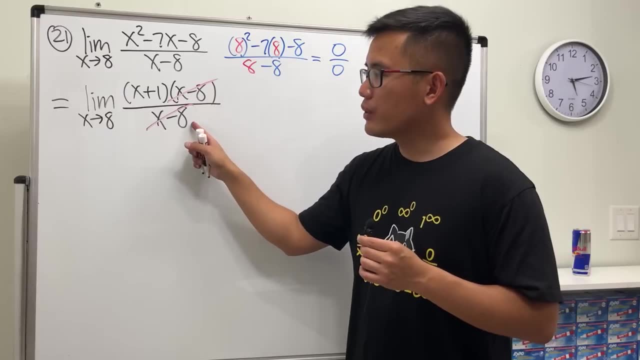 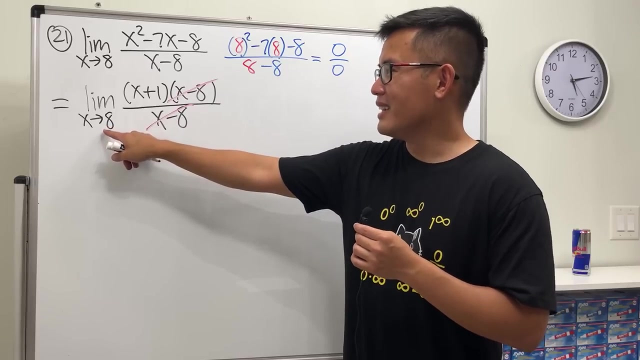 over, x minus 8.. have a look: x minus 8, x minus 8. cancel out so nicely. and once you cancel out this common factor, then you wouldn't get a 0 over 0 anymore, because you can see when we put the 8 in. 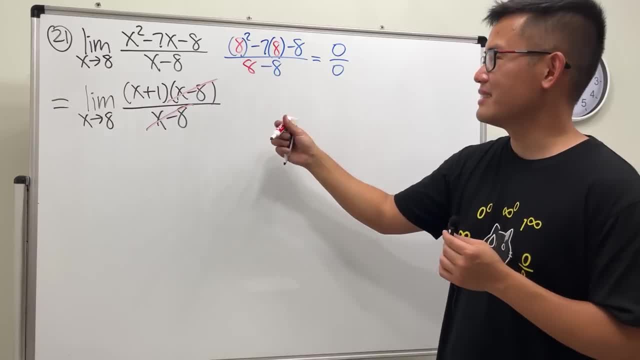 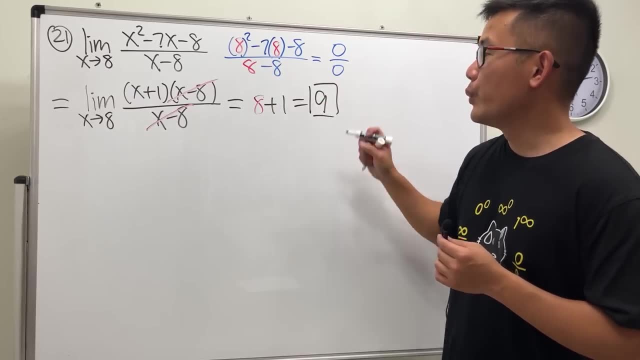 here: 8 plus 1.. nice number, that's the nice answer. you can see when we put the 8 in here: 8 plus 1.. nice number, that's the nice answer. so now just go ahead. i'll show you guys the work: 8 plus 1, so the answer is 9, and then we are done. 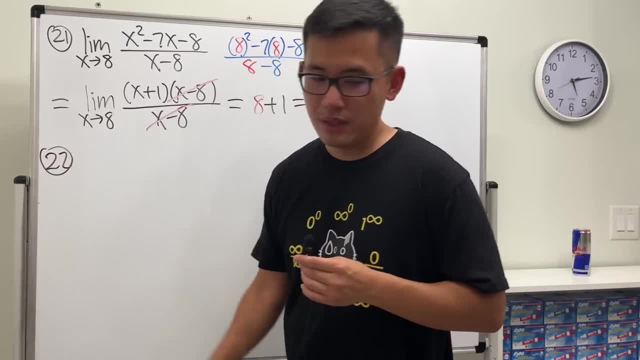 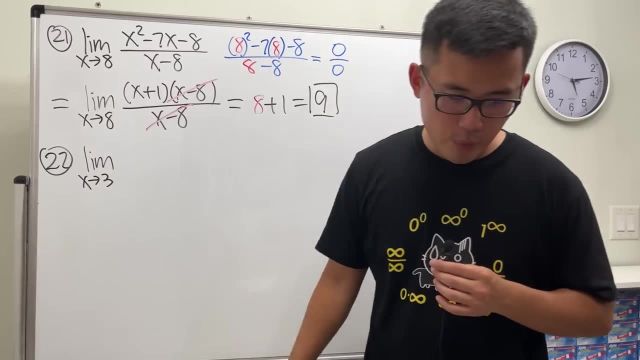 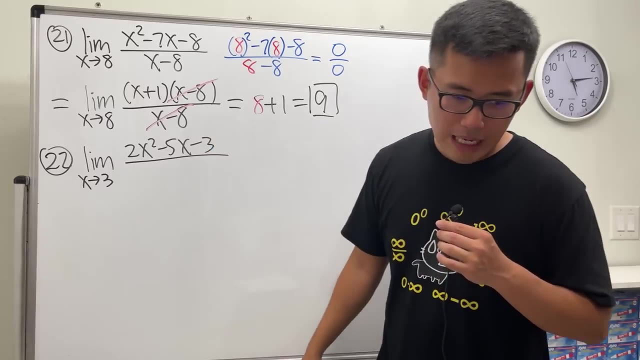 okay, so that's the answer for that. all right, number 22: let's see the limit as x approaches 3, and then we have 2x squared minus 5x minus 3, and on the bottom we have x square minus 2x minus. 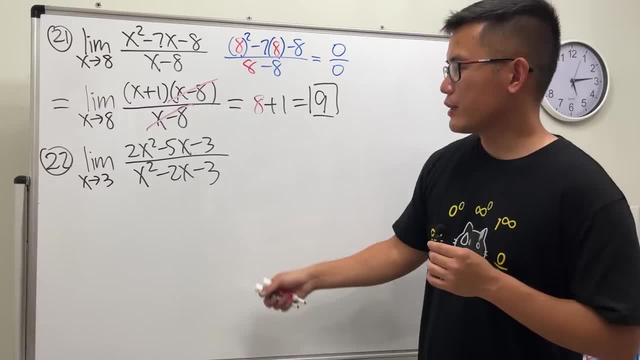 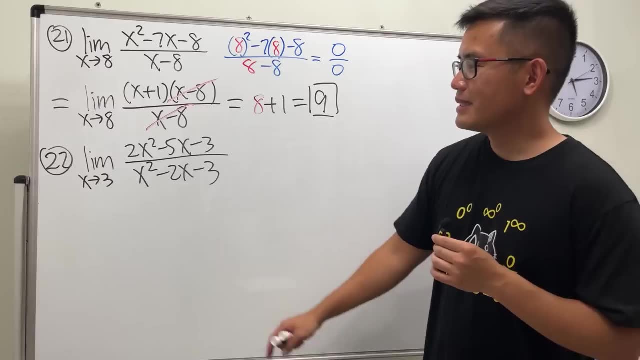 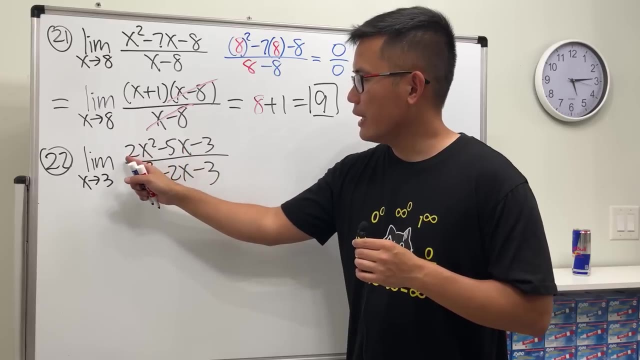 three, all right. so again, you should have a good habit that plugging the string to all the X's. you can work this out on your own. for you see, three in here is nine times size 18, that's 15. so 18 minus 15 is 3. 3 minus 3 we get 0. 9 minus 6 is 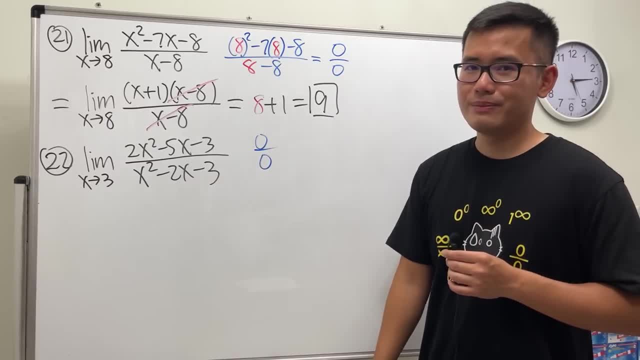 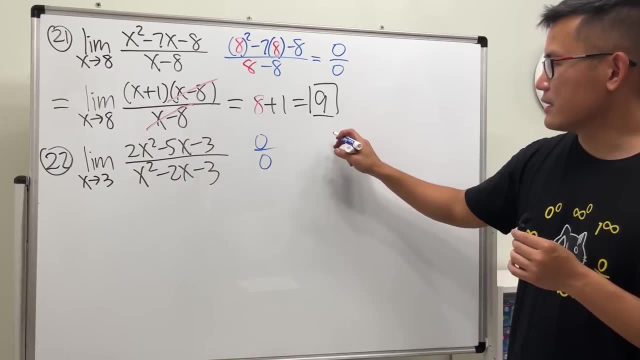 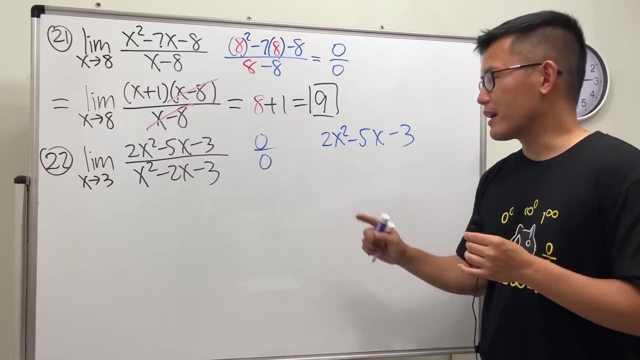 3 minus 3 is 0. so yeah, 0 over 0. do more work for this trinomial. trinomial, we can factor it. I'll show you guys how to factor this guy on the side 2x squared minus 5x minus 3. it's usually a little bit harder to factor when we have a 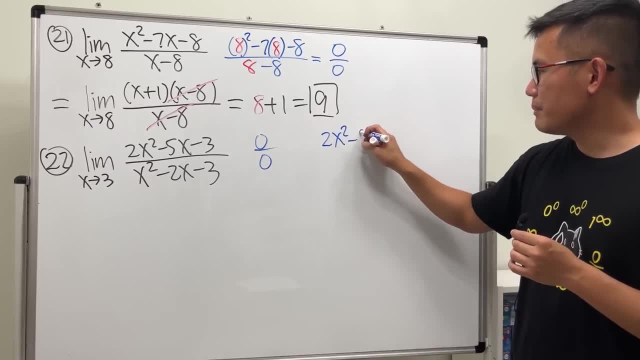 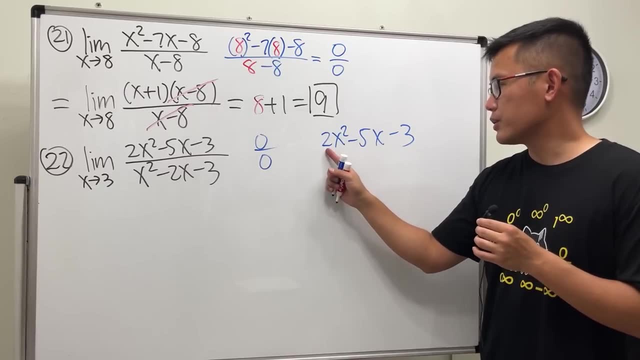 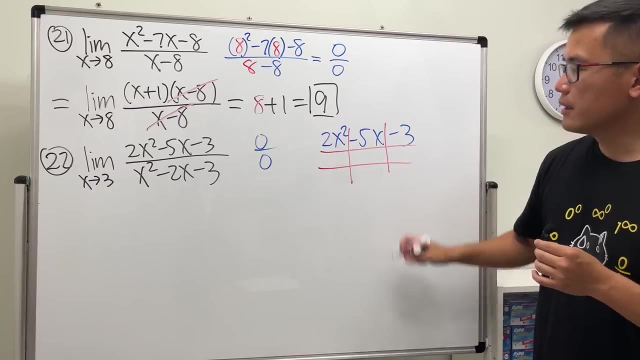 guys how to factor this guy on the side 2x squared minus 5x minus 3. it's usually a little bit harder to factor when we have a number that's not 1 in front of the x square, so I prefer to show my students the tic-tac-toe method. you just 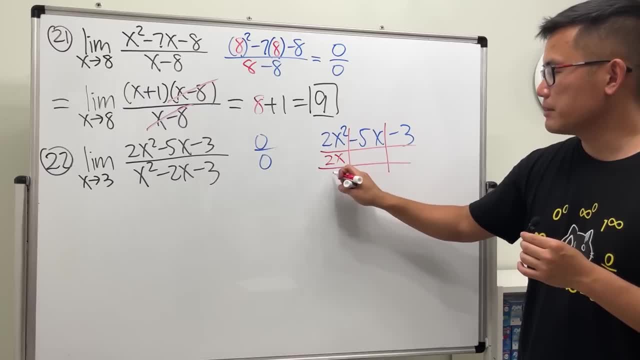 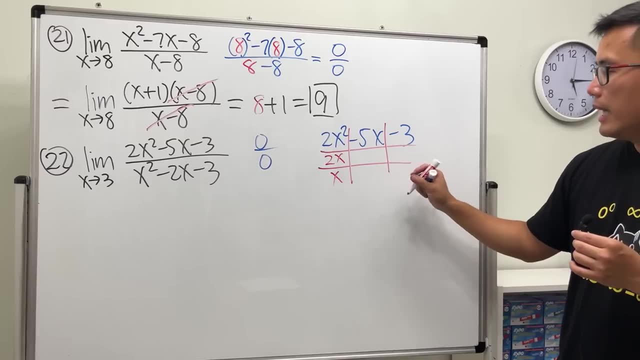 ask yourself: what times? what give you 2x squared? and the combination is 2x times X. and then you come here and then you ask yourself: what times? what give you negative 3? and it wouldn't matters, I'm going to put negative 3 here and 1 here. 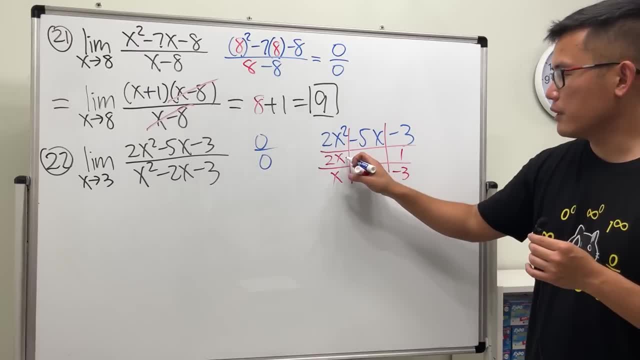 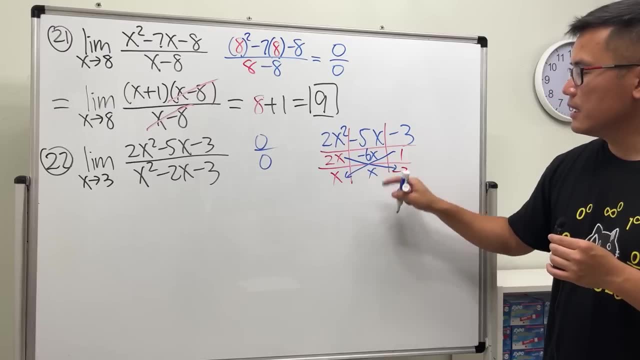 this works because now we can do the check and I can convince you: 2x times negative. 3 gives us negative. 6x 1 times X gives us X in the middle. this is where you check negative 6x plus X does give us negative. 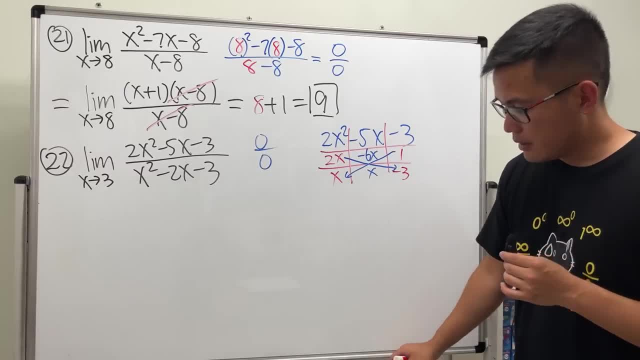 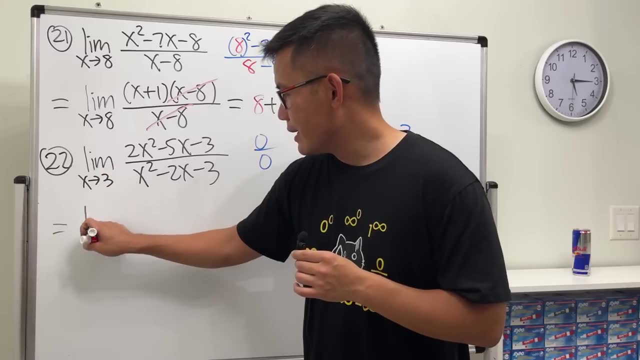 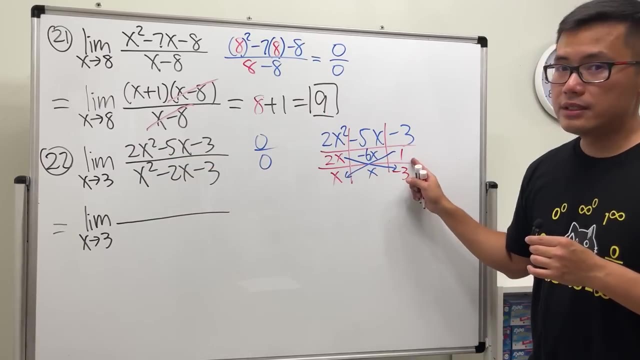 5x. so this is the correct factoring. we have found our correct combination, but this is how you're going to write down the answer for the factoring, wise. anyway, here we have the limit X approaching 3 on the top here. read this across, so we. 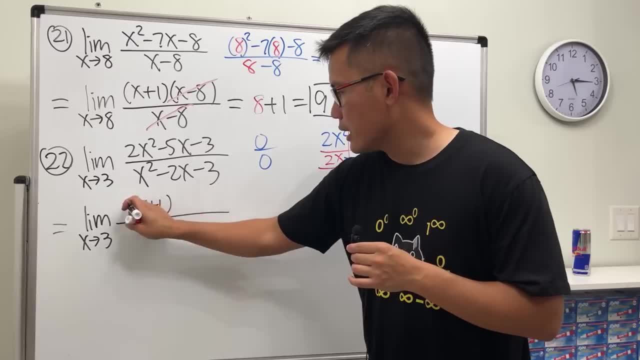 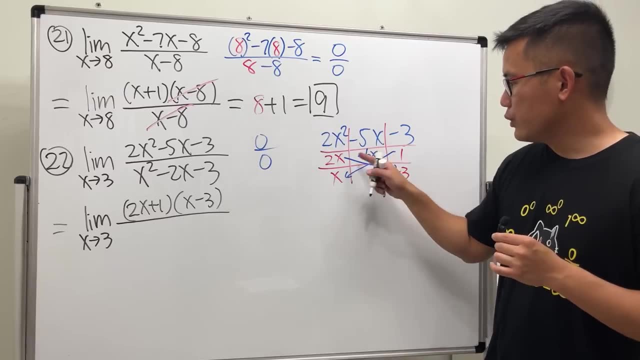 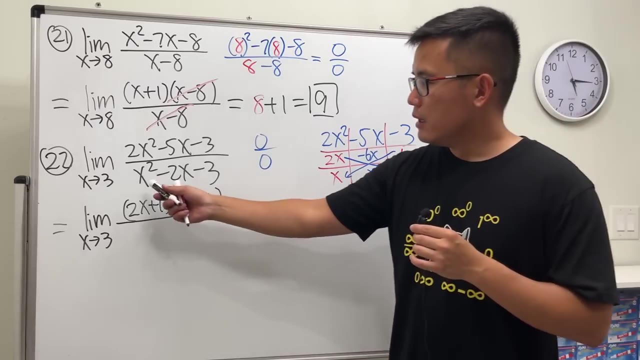 first have 2 X plus 1 and then bottom is X minus 3, right? so that's the factoring. you cross, multiply to check and then you really across like 2x plus 1, x minus 3. that's for the answer for this. right here you can factor the usual way, right, just like. 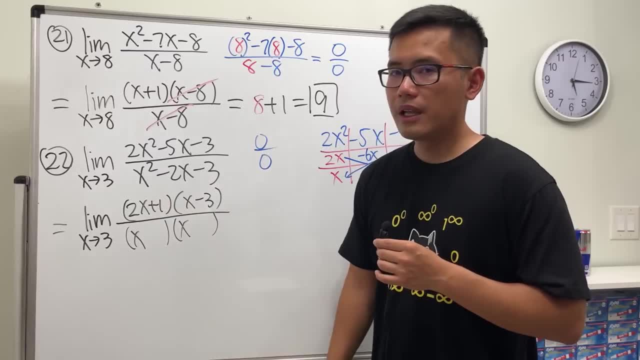 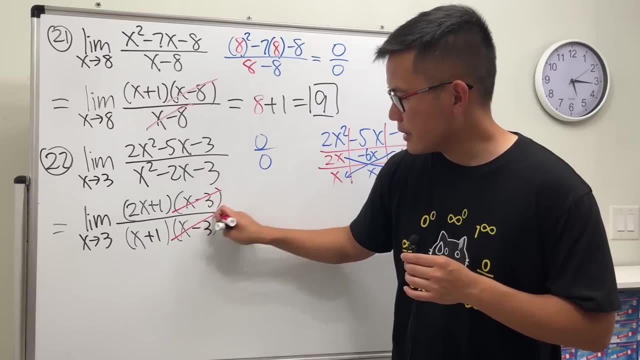 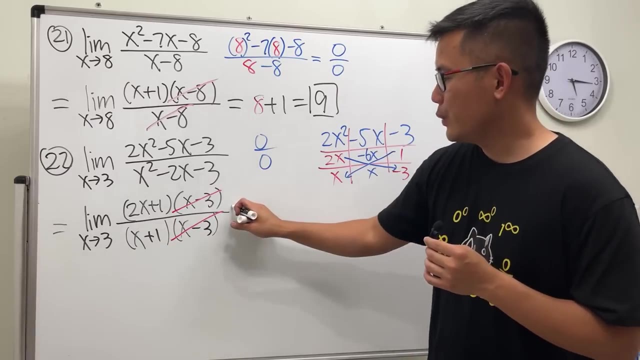 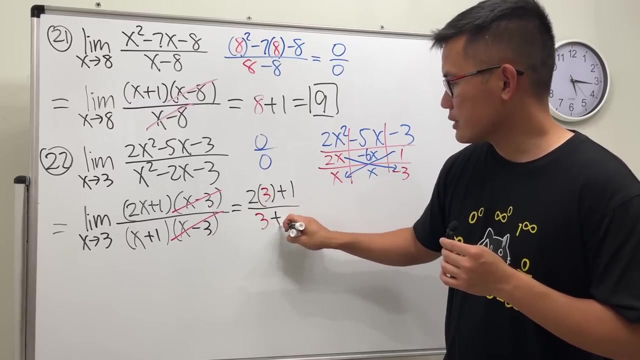 x times x, give us x square, and then we need plus 1 and then minus 3 to make this happen. and you see it: x minus 3, x minus 3, cancel. and then we can just put a 2- sorry, we can just put a 3- into this and that, and it worked out, and we will get 2 times 3 plus 1 over 3 plus 1, that's 7. 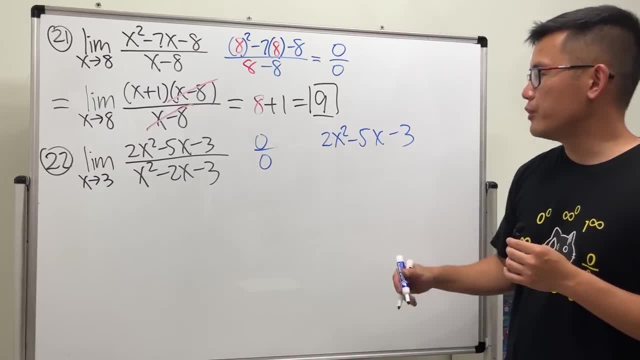 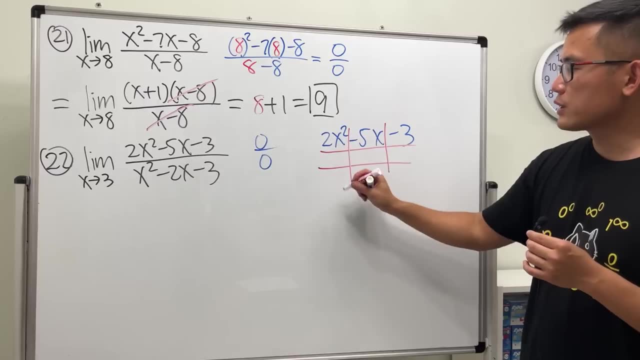 number, that's not 1, in front of the x square. so I prefer to show my students the tic-tac-toe method. you just ask yourself what times will give you 2x squared, and the combination is 2x times X. and then you come here and then you ask: 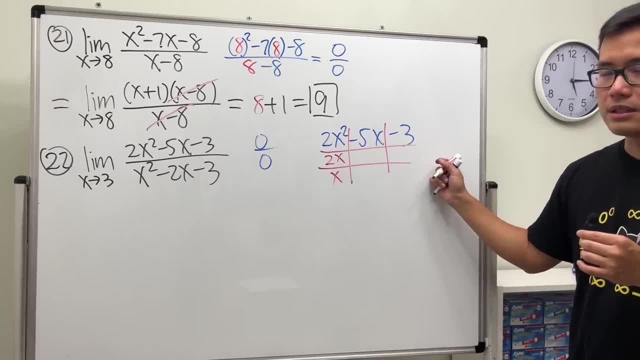 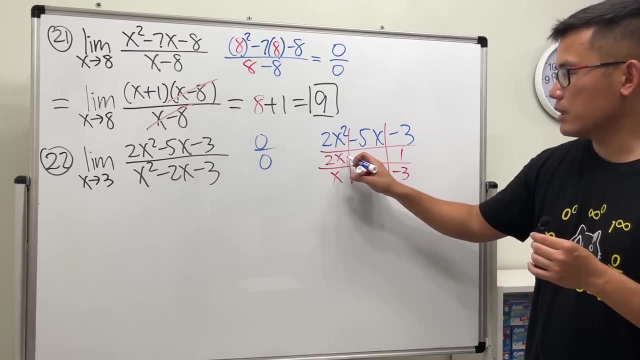 yourself what times will give you negative 3, and the water matters. I'm going to put negative 3 here and 1 here. this works because now we can do the check and I can convince you 2x times negative 3 gives us negative 6x 1 times. 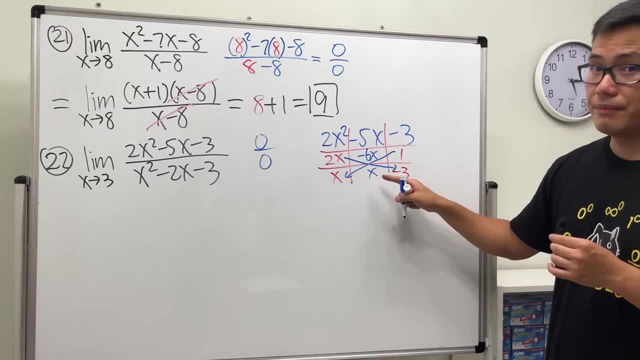 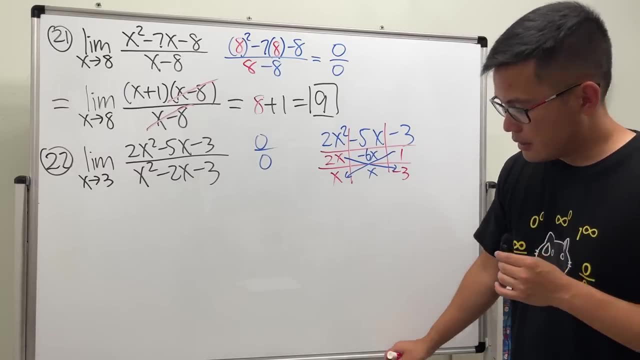 X gives us X in the middle. this is where you check negative 6x, plus X does give us negative 5x. so this is the correct factor in factoring. we have found our correct combination. but this is how you're going to write: only answer for the factoring wise anyway. 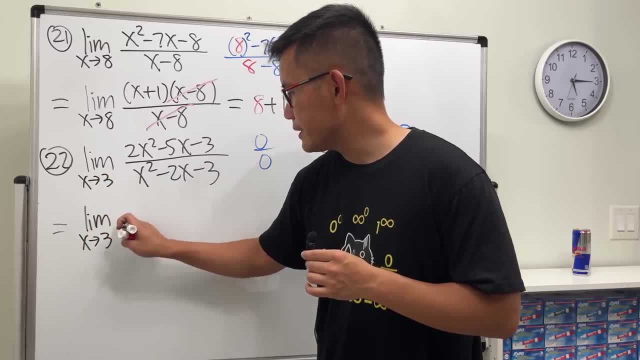 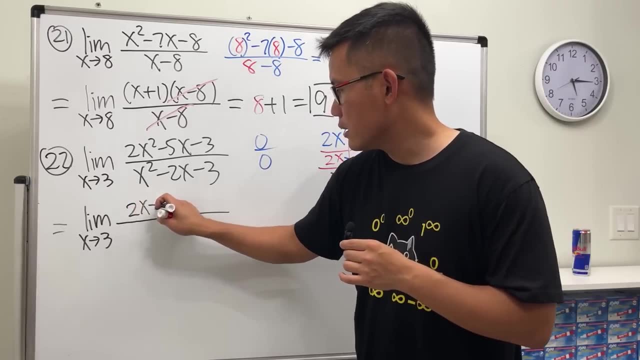 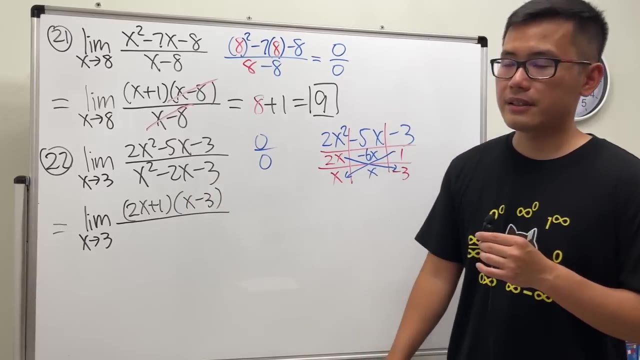 here we have the limit X approaching 3 on the top. here readies across so we first have 2x plus one and then bottom is X minus three. all right, so that's the factoring. you cross multiply to check and then you read across like two X plus one plus X minus three. F轉 derby describe cross and jjon lik 0x1 31008. Dad was lasciaoh 2 x2 По Fa charity. you cross multiplied to: check and you'll read it across like 2x plus one. then if you & X, 0, 0 after thatNOs you cross, multiply to, you cross, multiply to check, and then you will write A acrostic. you cross, multiply to check and then you really uh, cross. our cheapest реш grupo will force Friend learning opportunities, which means we'll express how we're talking about. 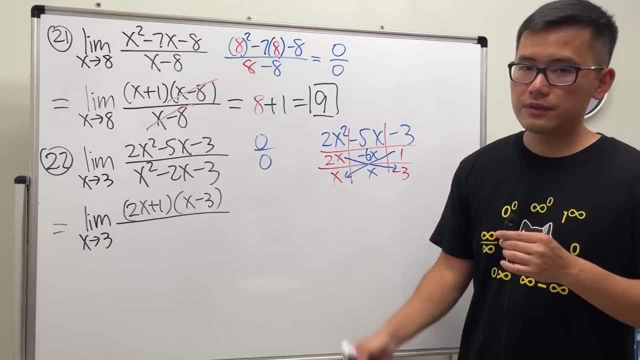 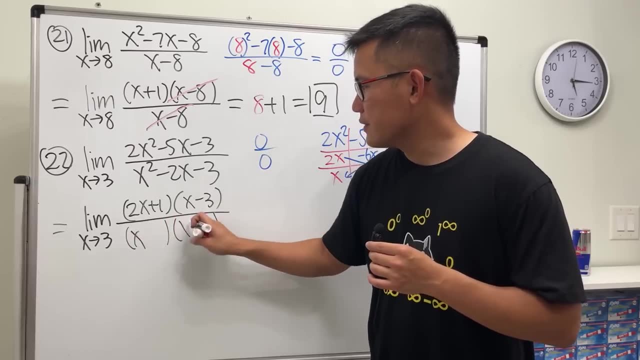 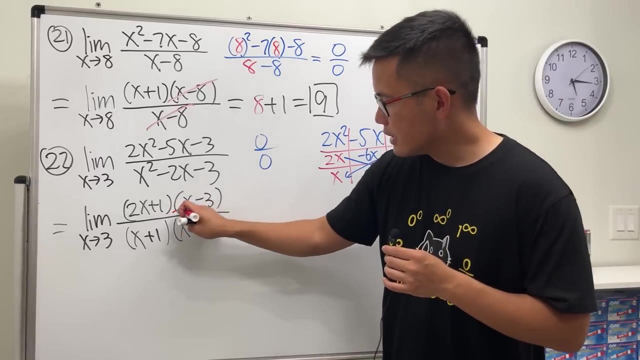 really across like 2x plus 1, x minus 3. that's for the answer for this. right here you can factor the usual way, right, just like: x times x give us x square, and then we need plus 1 and then minus 3 to make this happen and you see it: x minus 3, x minus 3, cancel, and then we can just put a 2. 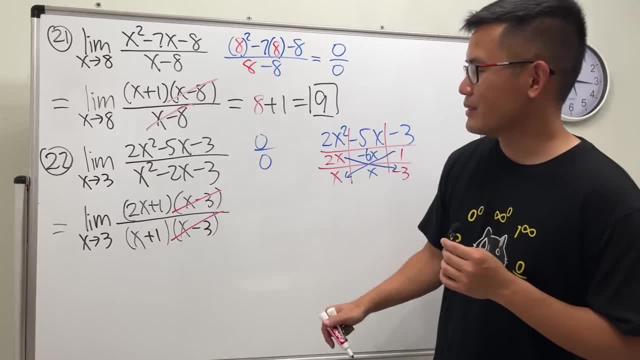 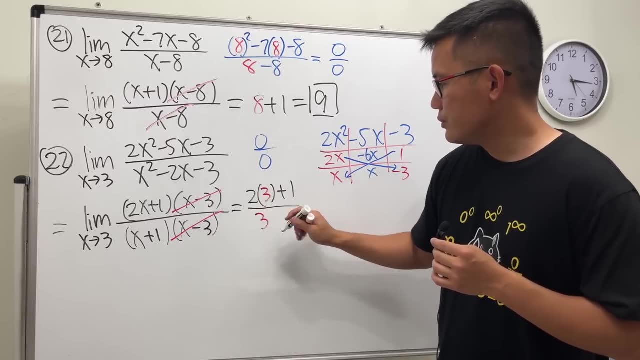 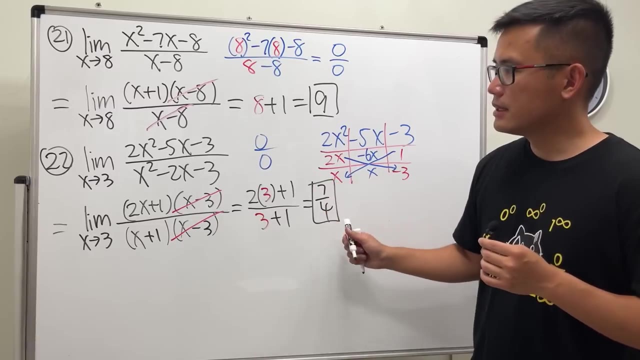 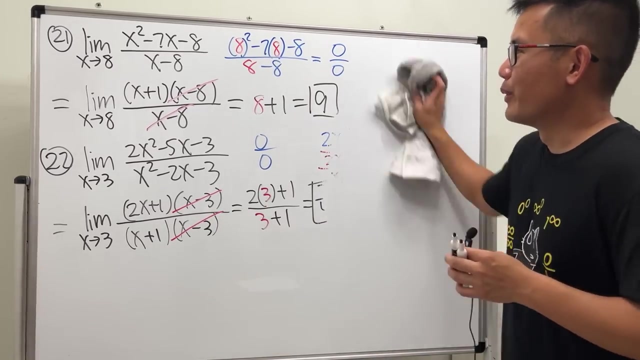 sorry, we can just put a 3 into this and that and it worked out, and we will get 2 times 3 plus 1 over 3 plus 1. that's 7, that's 4, so altogether 7 over 4 done, yay, all, right now i'm going to erase the board. 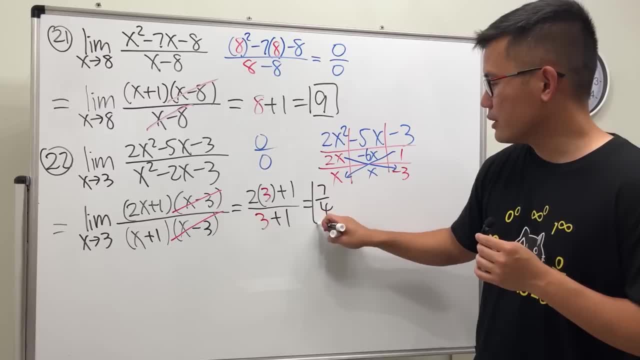 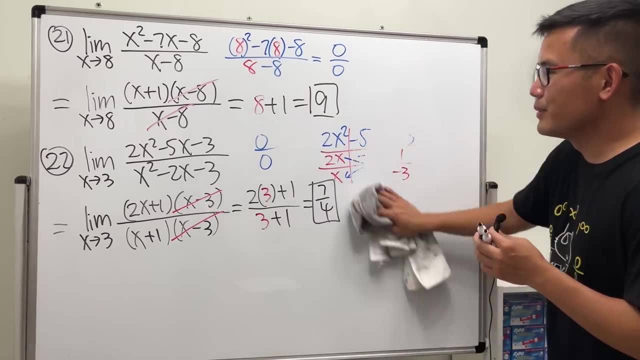 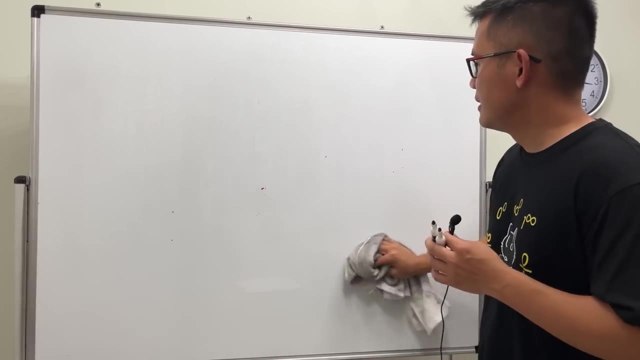 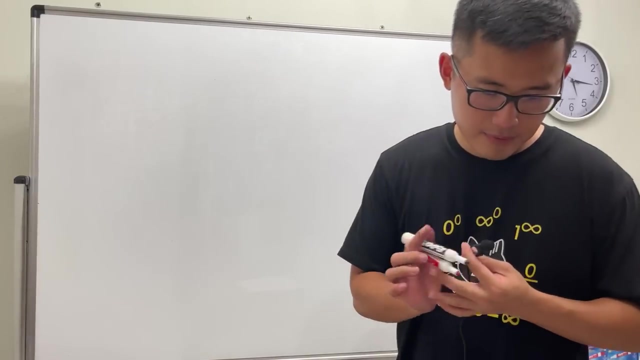 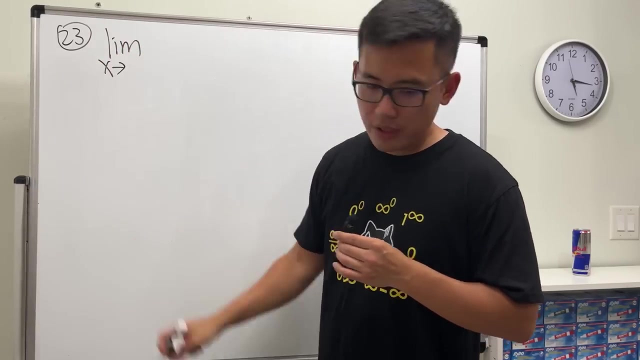 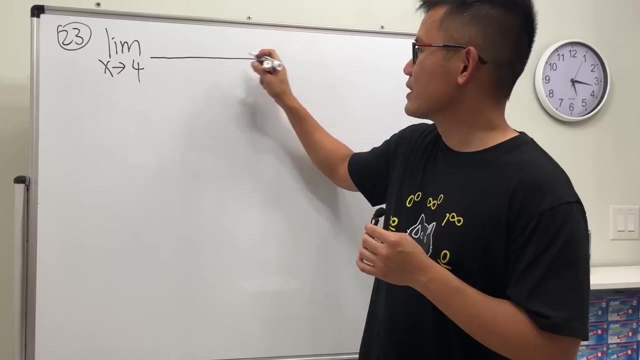 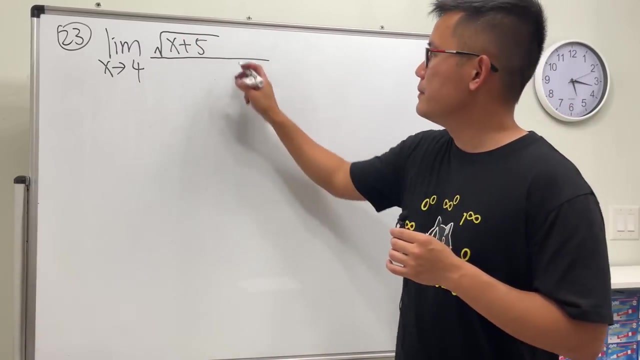 that's 4, so altogether 7 over 4 done, yay, all, right, now i'm going to erase the board number 23. here we have the limit as x approaching 127- no, just kidding- x approaching 4, and then we have a square root: x plus 5 and then minus 3, and then minus 3 is outside of. 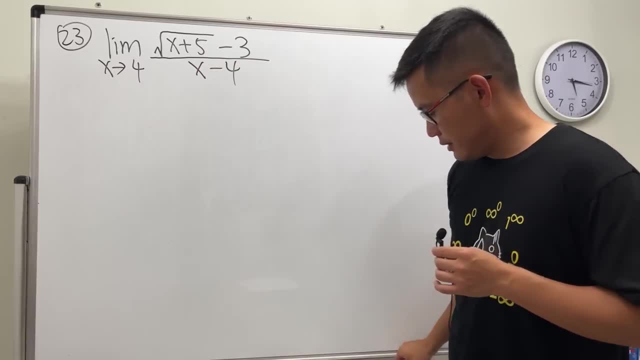 square root and i'm going to put it in the middle, and then minus 3 is outside of square root and bottom we have X minus 4.. All right, have a good habit Plugging 4 into here. 4 plus 5 is 9.. Take: 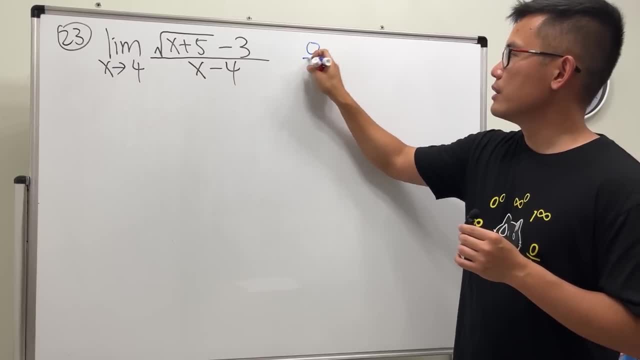 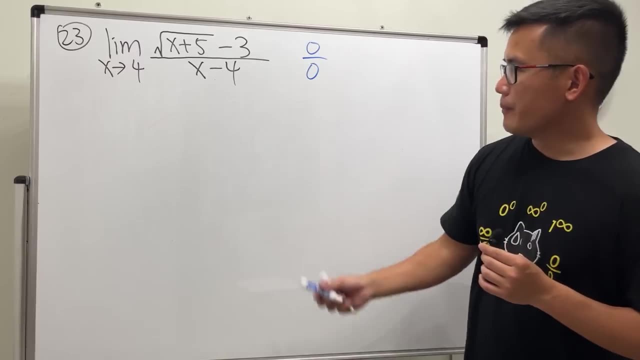 the square root of that is 3.. 3 minus 3, we get 0.. 4 minus 4 is 0. 0 over 0 situation. We have to do more work. Here's the deal. When we have a square root, it seems that we cannot factor the usual. 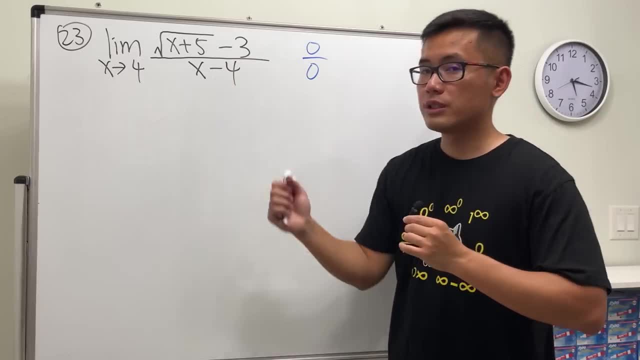 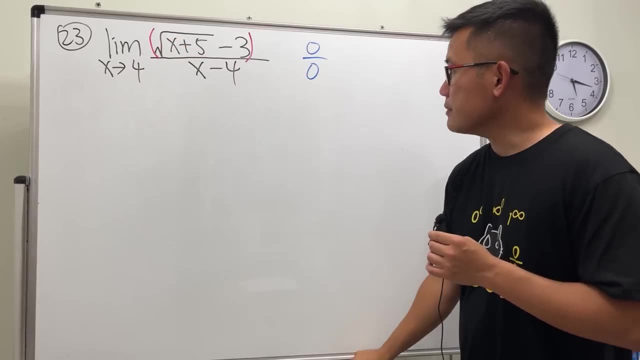 way. However, when we have a square root expression like so, we can use the conjugate to help us simplify it, And by that we mean to multiply the top by and again. let me just put a 0 over 0. 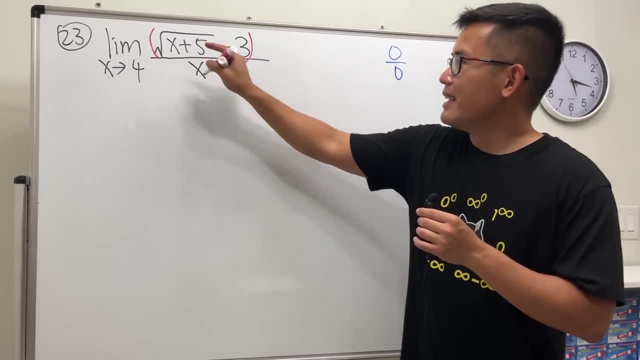 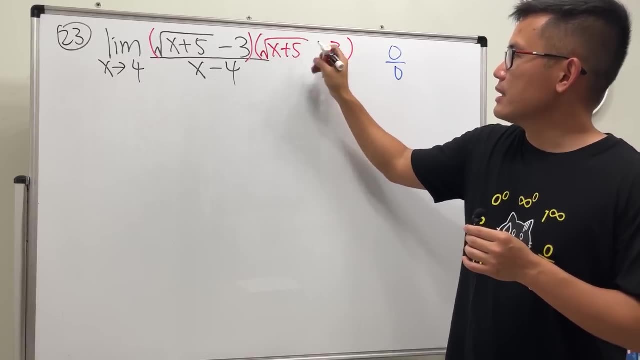 all the way here. All right, I'm going to keep this and that, So we have square root of X plus 5 and then 3.. But instead of the minus, we are going to put a plus in the middle. And, of course, 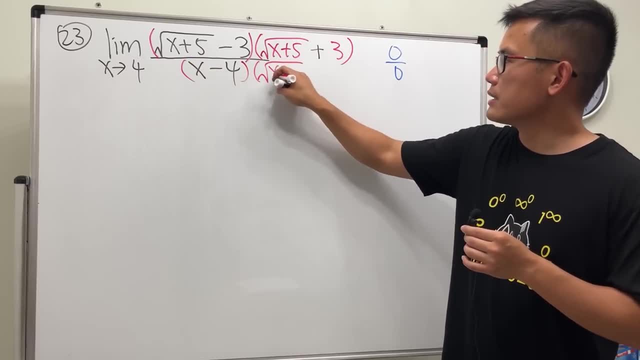 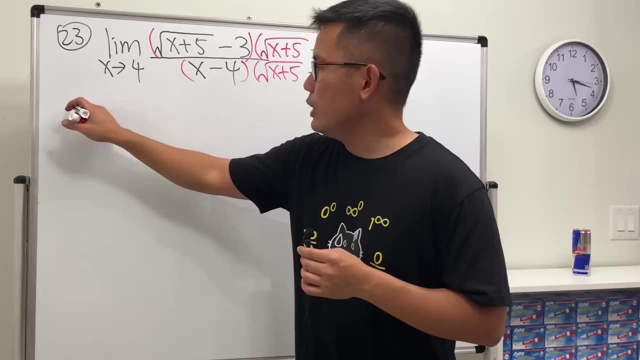 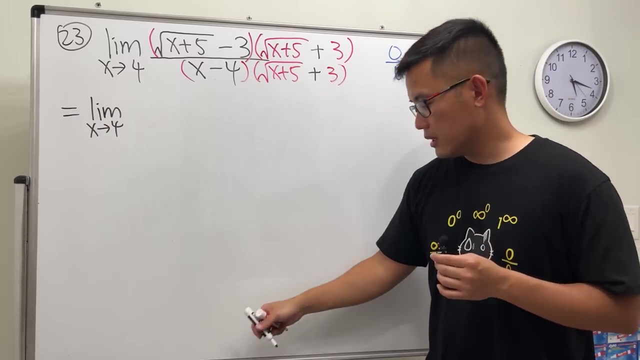 we do the same thing on the bottom, So square root of X plus 5 and then plus 3.. Okay, Okay, And now we can work this out relatively easily. When I say that, it's because when we multiply the conjugate, we have an easy way to do it. Here's the deal. When we are multiplying, 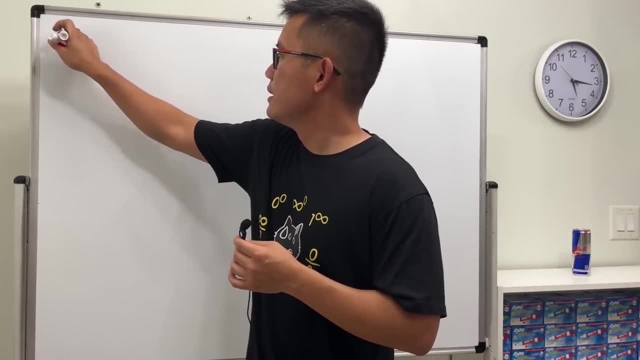 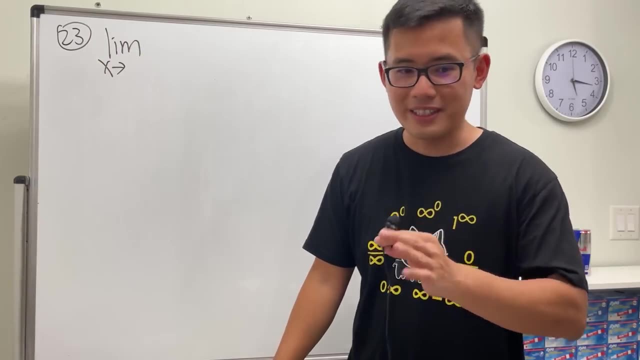 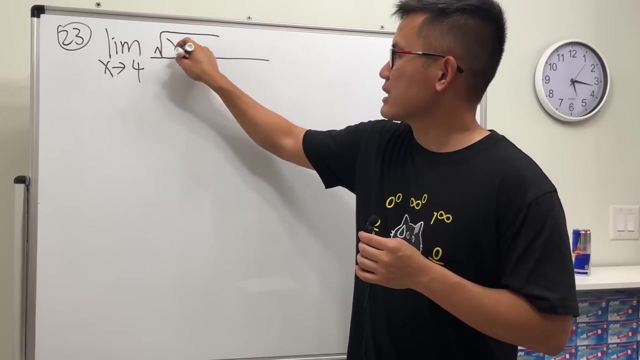 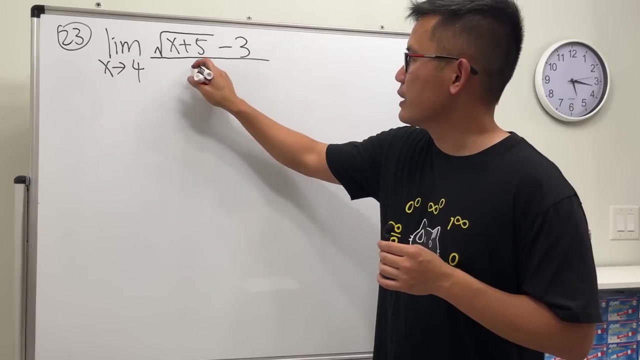 number 23. here we have the limit as x approaching 127- no, just kidding, x approaching 4, and then we have a square root: x plus 5 and then minus 3, and the minus 3 is outside the square root, and on the bottom we have x minus 4. all right, have a good habit. 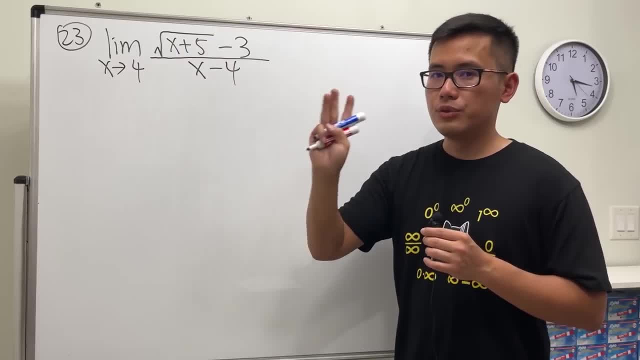 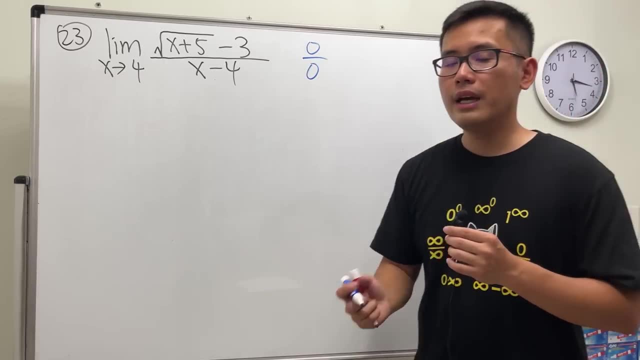 plugging 4 into here, 4 plus 5 is 9. take the square root of that is 3. 3 minus 3, we get 0. 4 minus 4 is 0. 0 over 0 situation. we have to do more work. here's the deal. when we have a square. 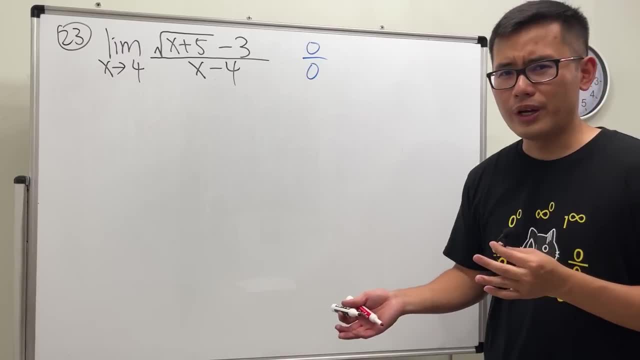 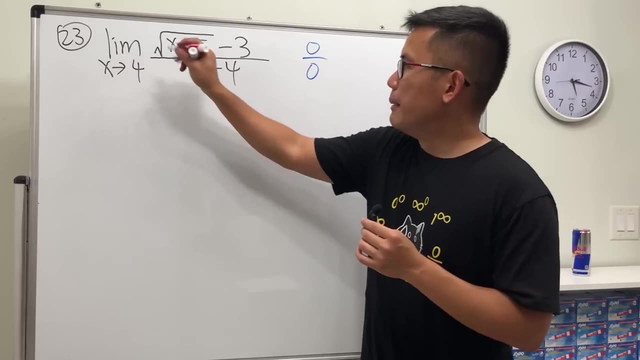 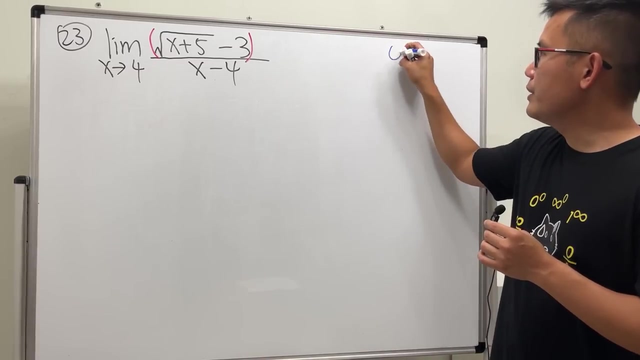 root, it seems that we cannot factor the usual way, huh. however, when we have a square expression like so, we can use the conjugate to help us simplify it, and by that we mean to multiply the top by 0. and again, let me just put a 0 for 0 all the way here. all right, i'm going to keep this and that so. 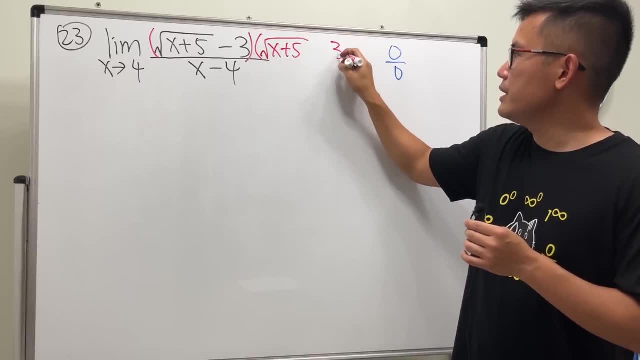 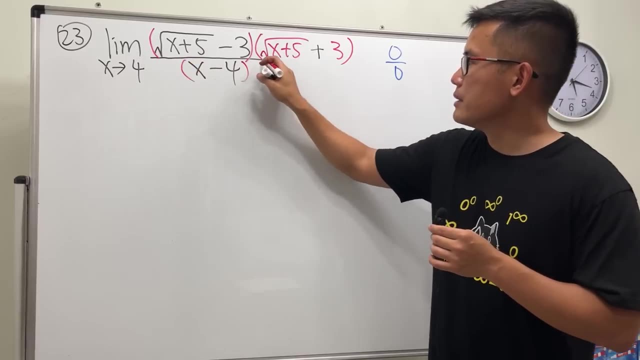 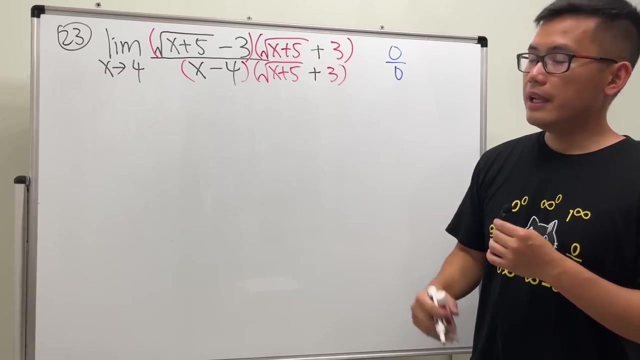 we have square root of x plus 5 and then 3, but instead of the minus we are going to put a plus in the middle and of course, we do the same thing on the bottom. so square root of x plus 5 and then plus 3. okay, and now we can work this out relatively easily when i say that we have a 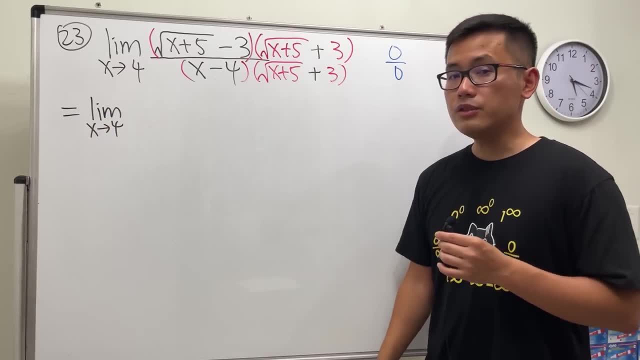 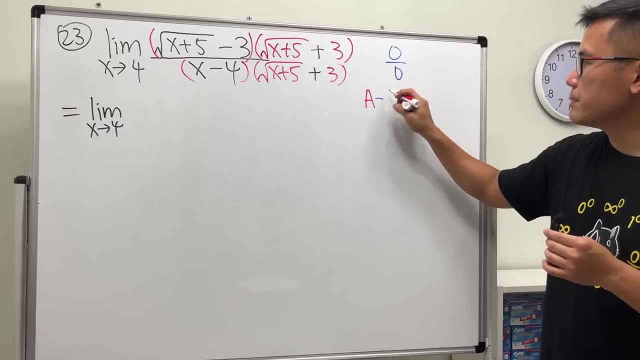 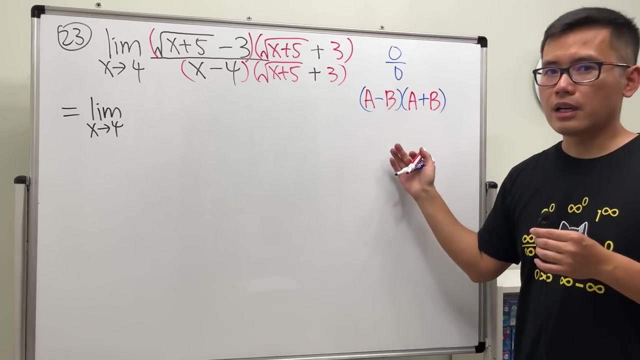 But it's because when we multiply the conjugate, we have an easy way to do it. Here's the deal: When we are multiplying a minus b times a plus b- and this is the purpose of the conjugate- you just change the sign in the middle. 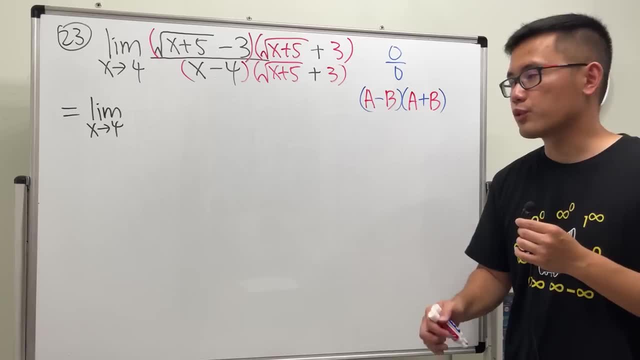 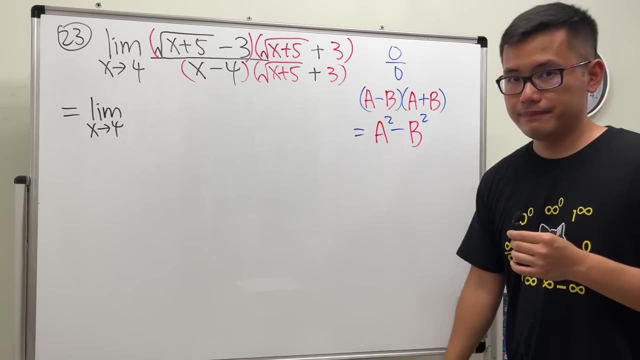 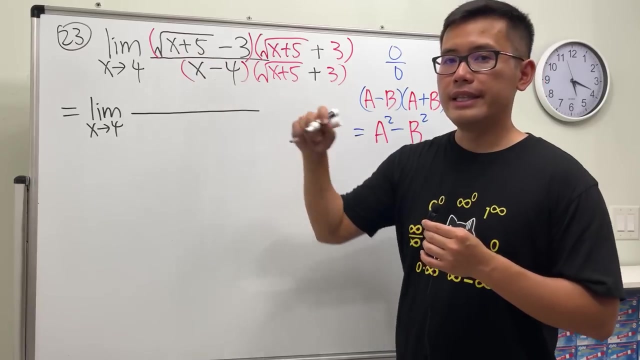 This right here: when we multiply, we actually just get a difference of two squares, Namely a squared minus b squared. So, coming back here, what we can do is just square the first thing and the square squared will cancel. 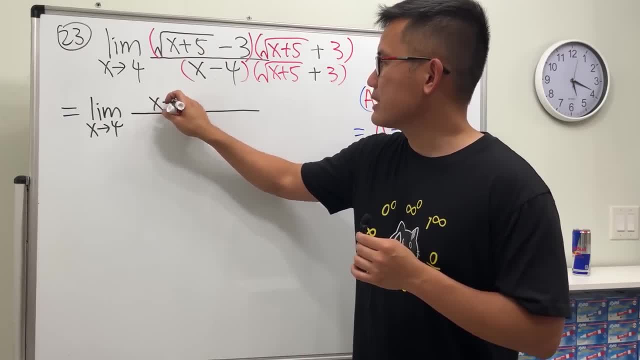 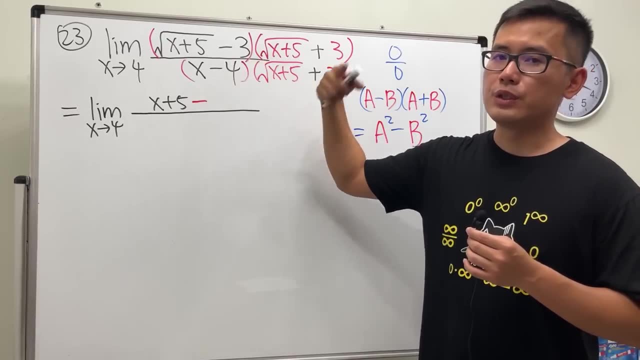 Perfect huh. So we get x plus 5. And then in the middle we have the minus, And then we look at the second thing, which is just a 3, and we square that 3 squared is a 9.. 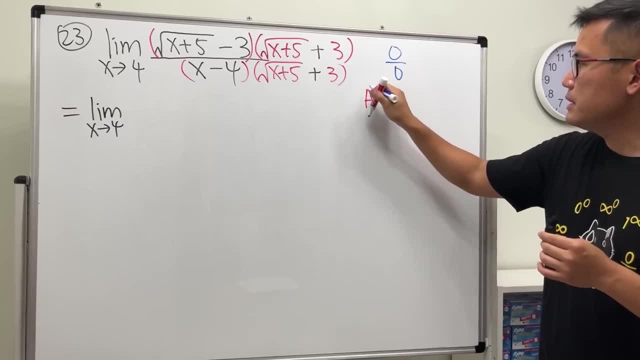 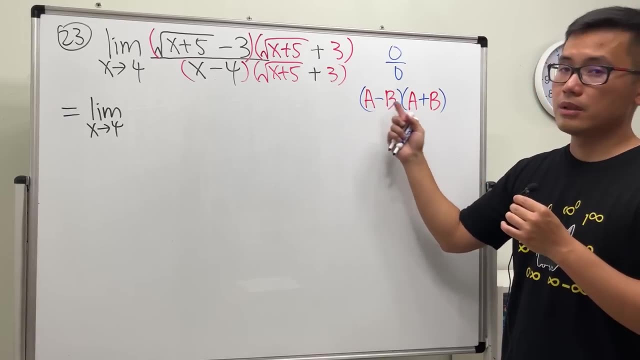 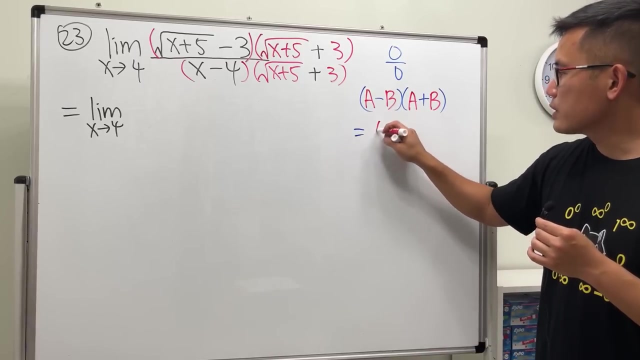 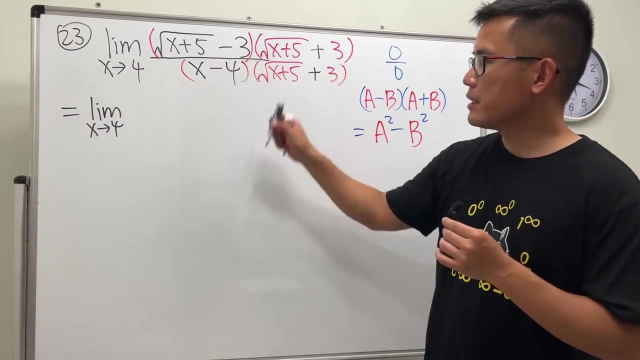 A minus B, times A plus B, And this is the purpose of the conjugate. You just change the sign in the middle. This right here. when we multiply, we actually just get a difference of two squares, Namely A squared minus B squared. So, coming back here, what we can do is just square the first. 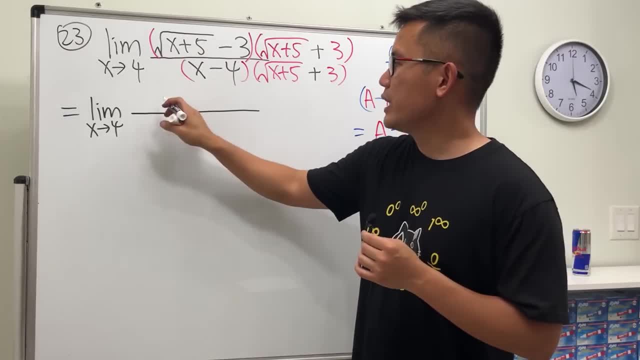 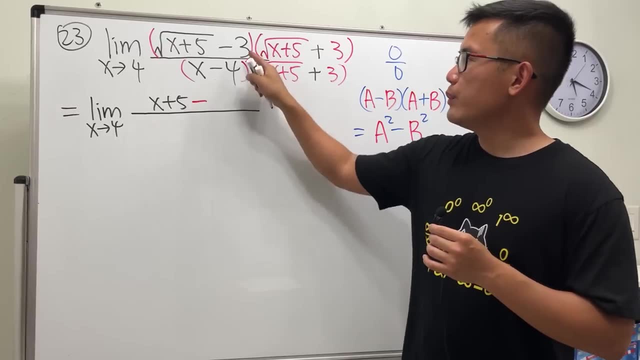 thing, and the square squared will cancel Perfect huh. So we get X plus 5. And then in the middle we have the minus. And then we look at the second thing, which is just a 3, and we square that 3. 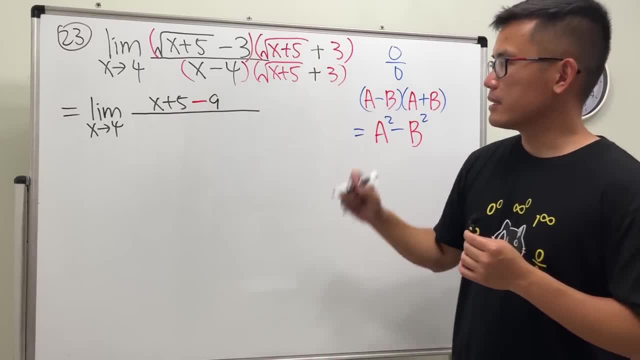 squared is a 9. Good, And on the bottom we have the minus. And then we look at the second thing, which is just a 9. Good, And on the bottom don't multiply the out, Because the purpose of the 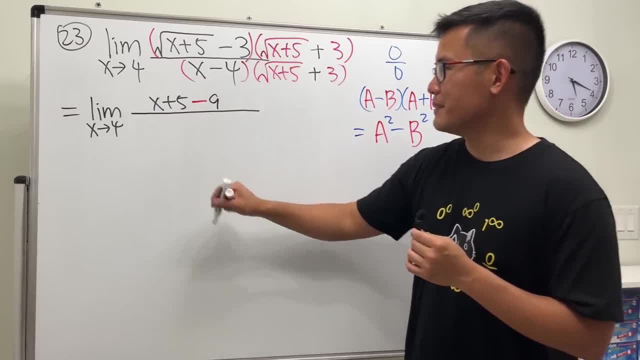 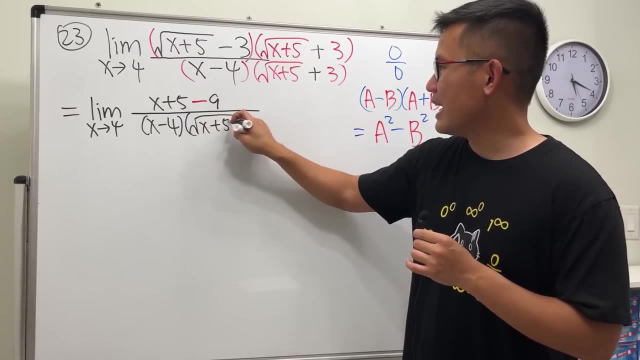 conjugate is to fix the top. Just keep the bottom as how it is and you'll see good things will happen. X minus 4 times all that, So square root of X plus 5 and then plus 3.. Now on the top. 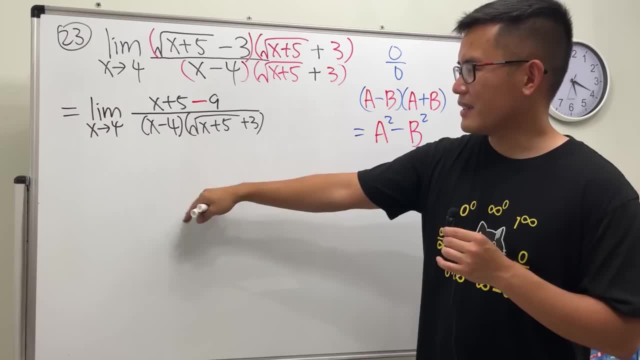 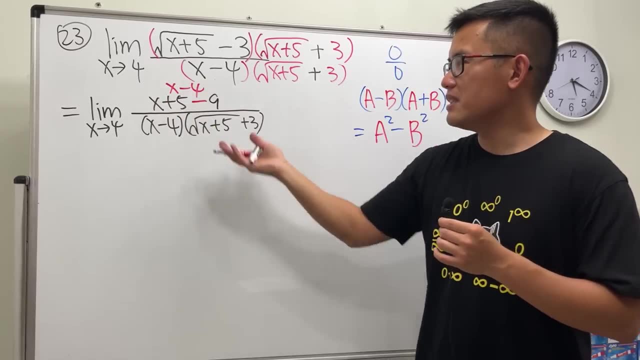 we have X plus 5 minus 9.. You don't have to write it down again and rewrite the whole thing. You can just write the result above and you'll see, this is just X minus 4.. Just be neat. and then this is: 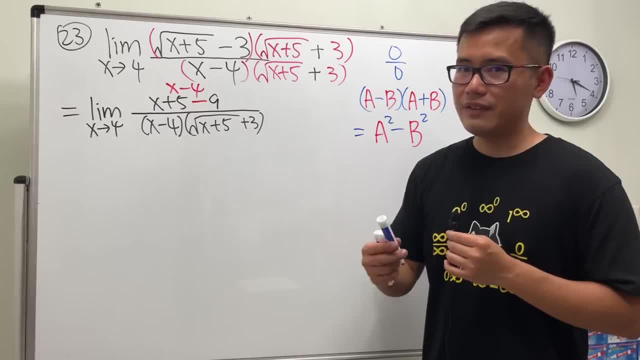 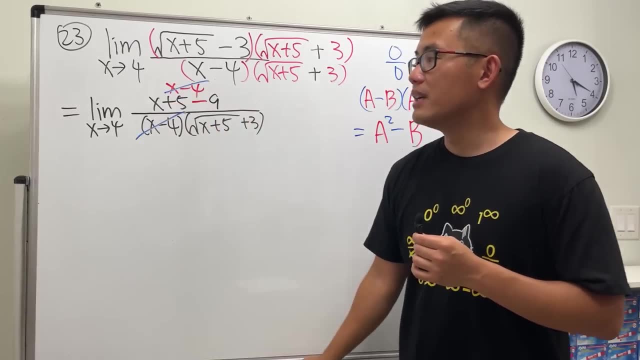 clear. And you see, on the top we just have X minus 4.. But guess what? On the bottom we also have X minus 4 as a factor. So this and that can be cancelled. And then, when we have that, well, we can now just 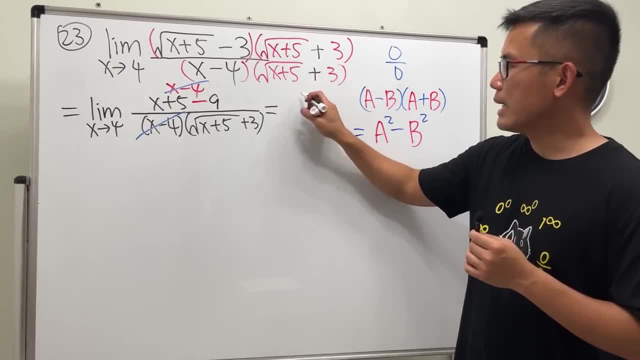 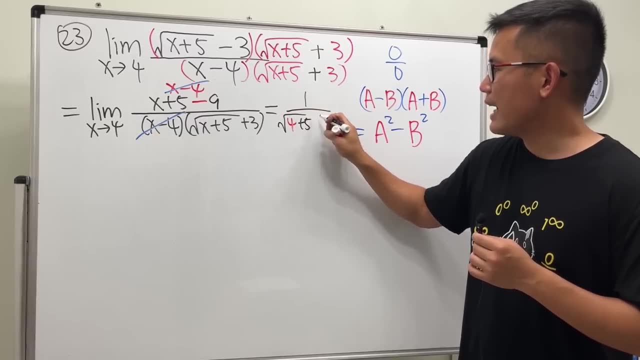 plug in the 4 into the X and work that out. So on the top we have 1.. That's cancelled. So we just have square root of 4 plus 5 and then plus 3. So only all we have. what 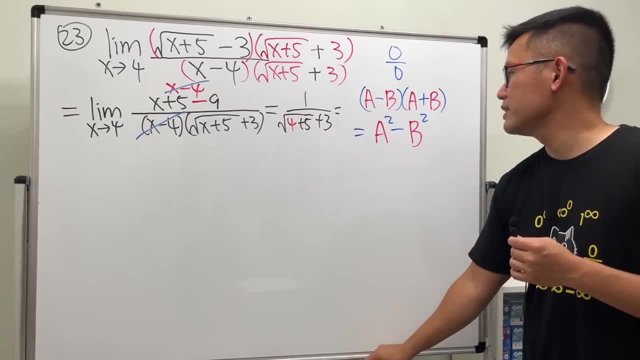 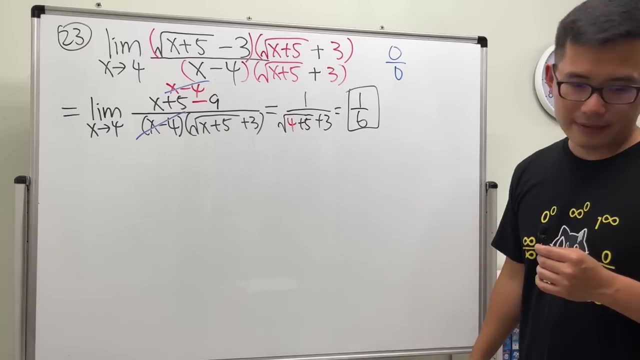 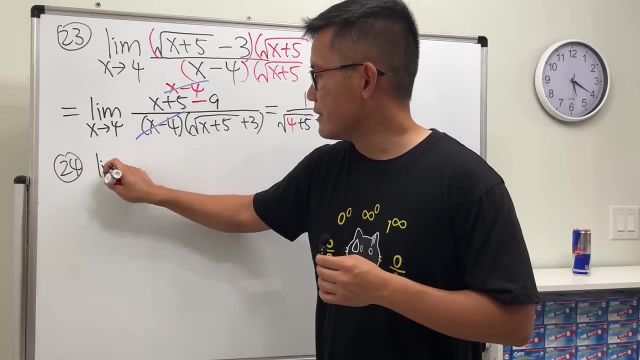 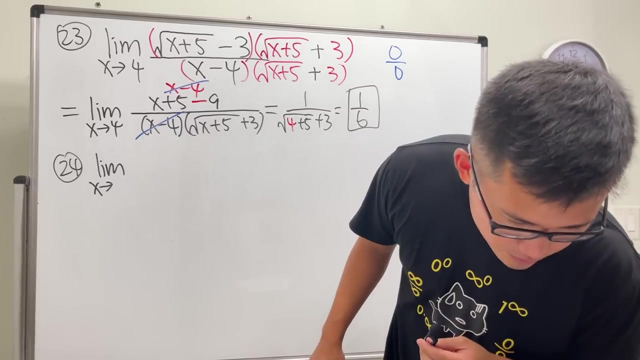 That's 3 plus 3.. So we have 1 over 6.. So that's the answer for that. Okay, number 24.. Here we have the limit as X approaching 2.. 2, 2.. All right, X squared minus 2X. 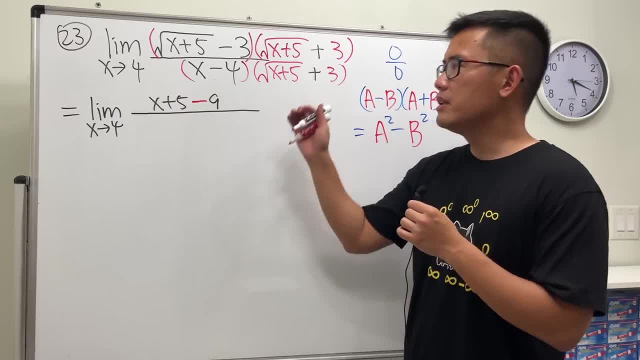 Good, Good, Good, Good, Good, Good. And on the bottom, don't multiply the out, because the purpose of the conjugate is to fix the top. Just keep the bottom as how it is and you'll see good things will happen. 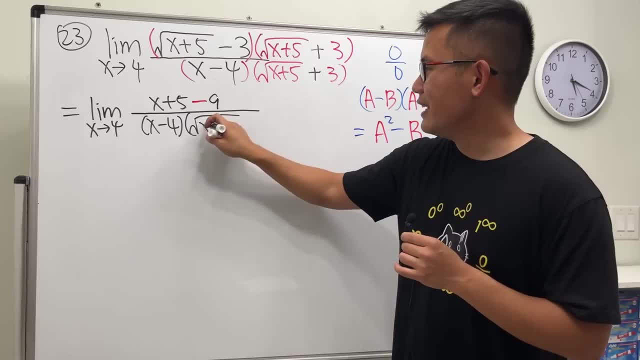 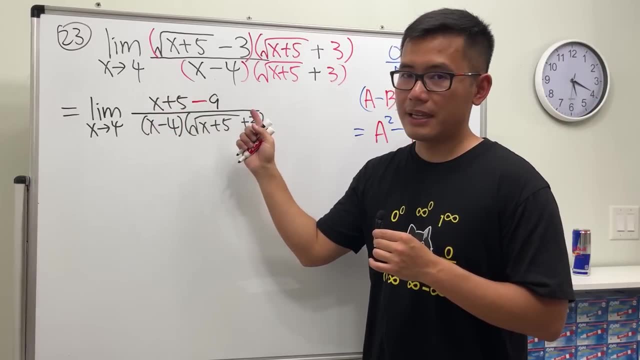 x minus 4 times all that. so square root of x plus 5, and then plus 3.. Now on the top we have x plus 5 minus 9.. You don't have to write it down again and I rewrite the whole thing. 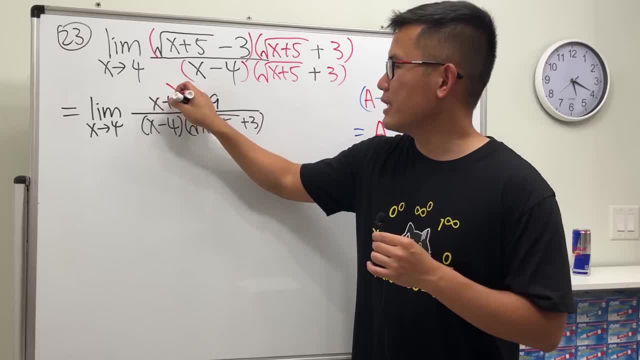 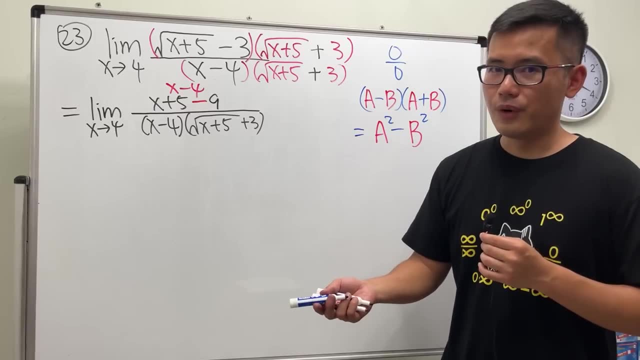 You can just write the result above and you'll see this is just x minus 4.. Just be neat. and then this is clear: And you see on the top we just have x minus 4.. But guess what? On the bottom we also have x minus 4 as a factor. 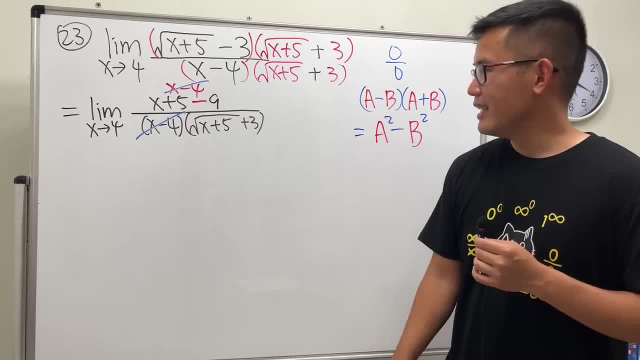 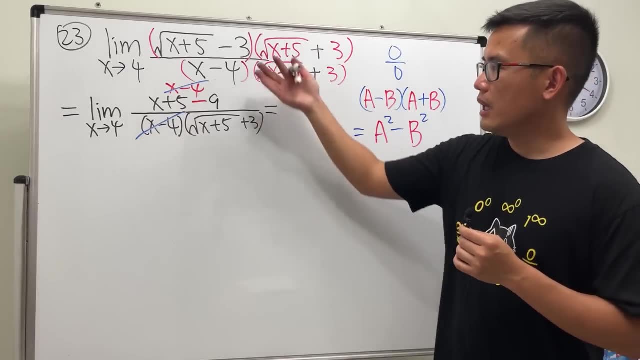 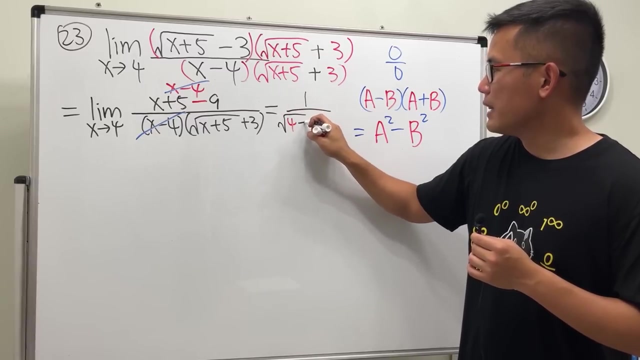 So this and that can be canceled. And then, when we have that well, we can now just plug in the 4 into the x and work that out. So on the top we have 1.. That's canceled it. so we just have square root of 4 plus 5, and then plus 3.. 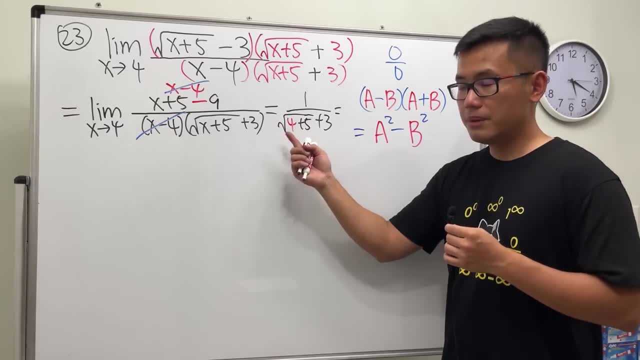 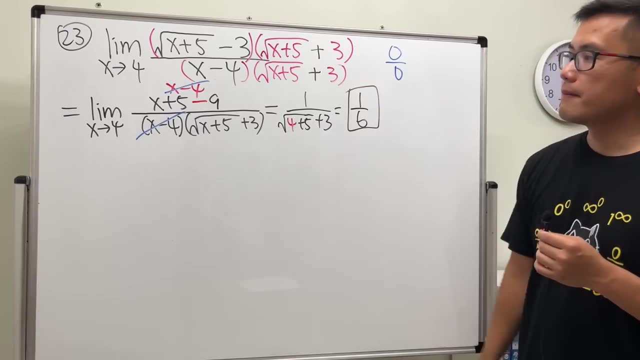 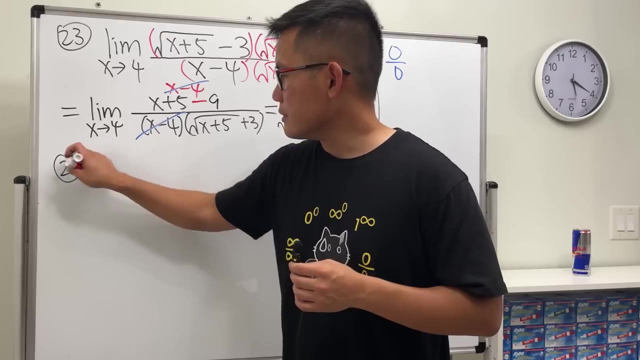 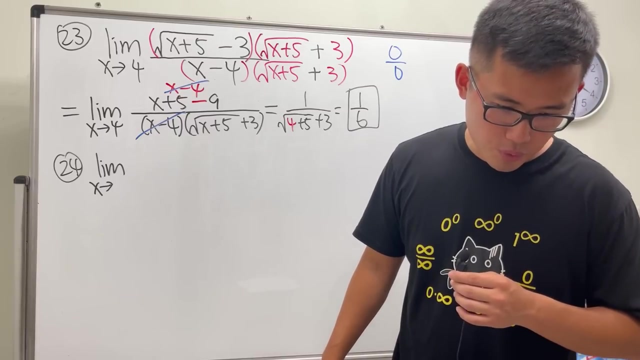 So all in all, we have x minus 4.. So we have what That's 3 plus 3,, so we have 1 over 6.. So that's the answer for that, OK, number 24.. Here we have the limit as x approaching 2.. 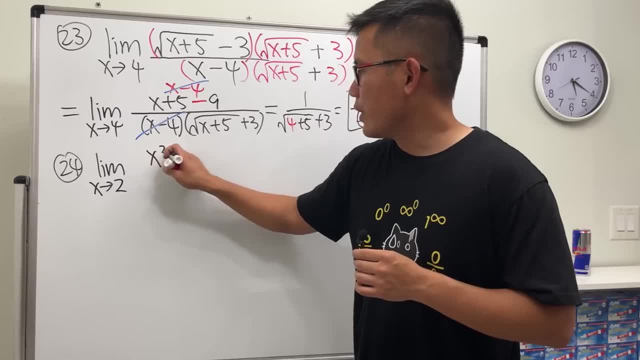 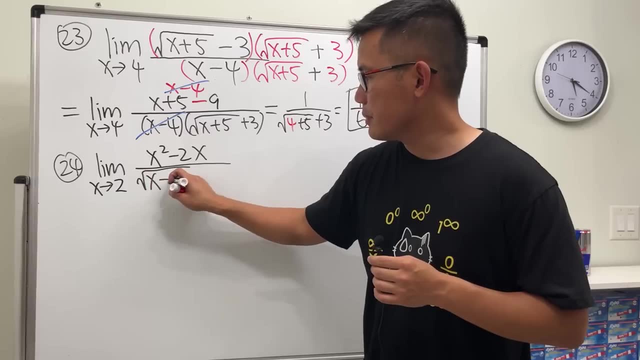 2, 2.. All right, x squared minus 2x. Over On the bottom we have a square root, So square root of x plus 2.. And then minus 2.. How many 2s do we have here? 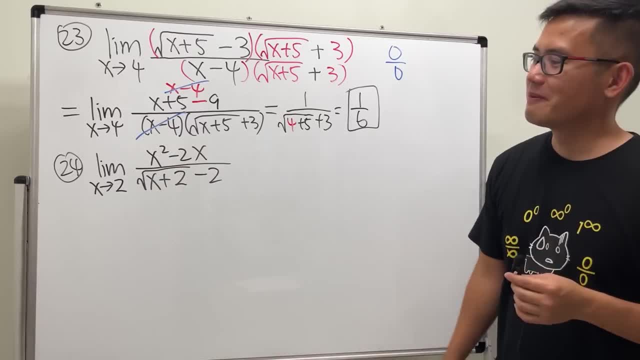 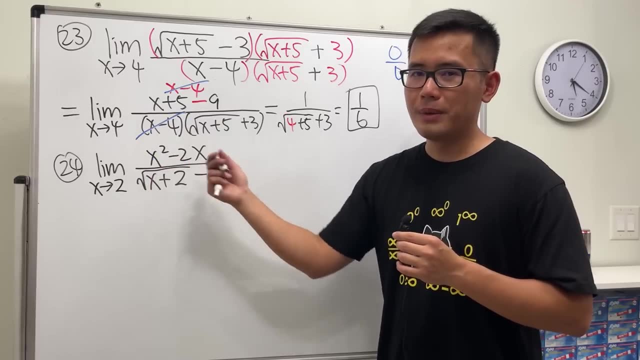 1, 2,, 3, 4, 5.. Anyway, have the good habit, Check this out. Put 2 in here and here. 2 squared is 4.. 2 times 2 is 4.. 4 minus 4 is 0.. 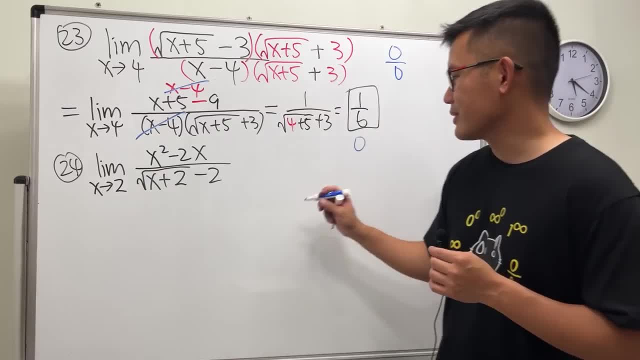 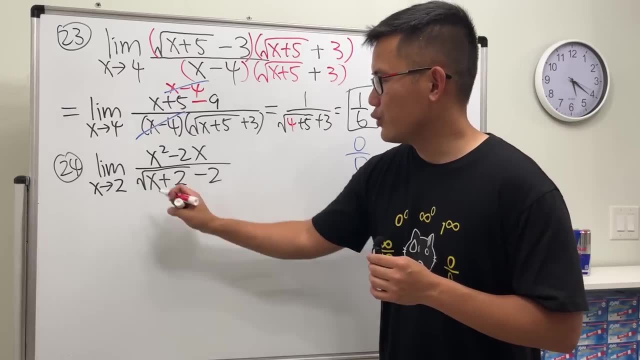 2 plus 2 is 4.. Square root of 4 is 2.. 2 minus 2 is 0.. So this is good. This is, yes, a 0 over 0 case. Don't worry, Can't you get again? fix the square root part first. 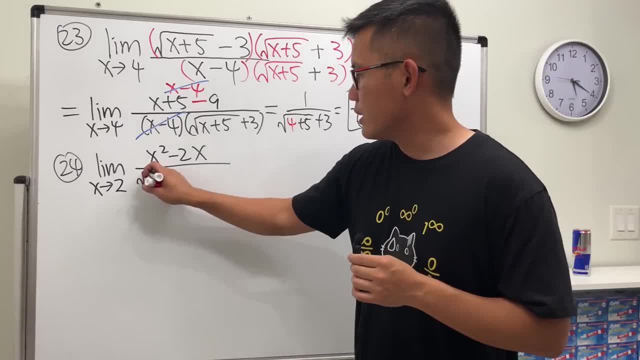 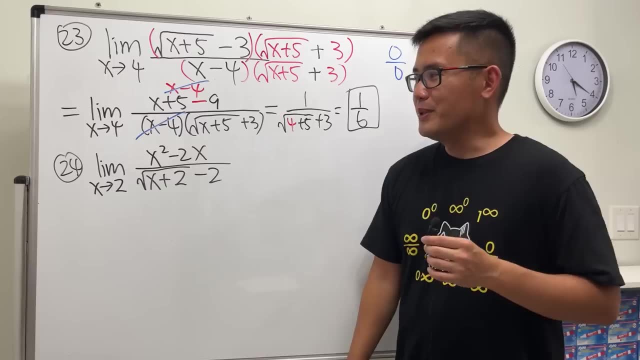 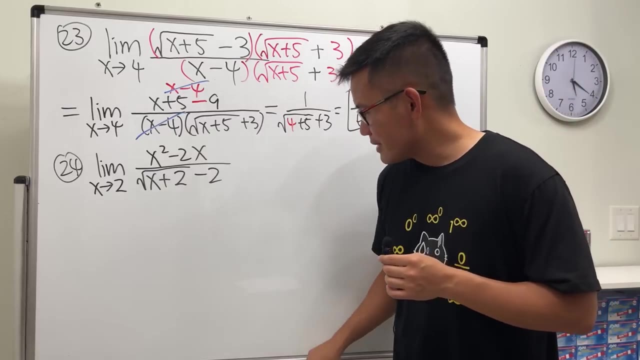 On the bottom we have a square root, So square root of X plus 2. And then minus 2.. Oh, how many 2s do we have here? 1, 2, 3, 4, 5.. Anyway, have the good habit, Check this out, Put 2 in here and 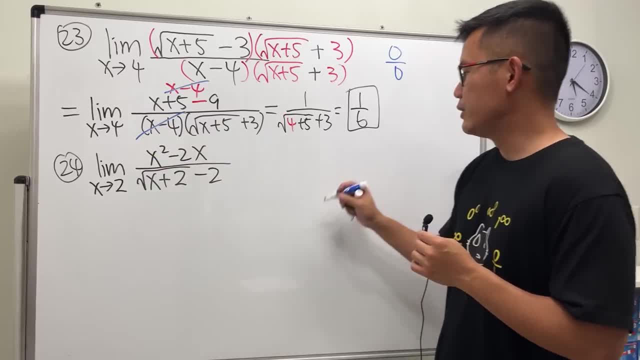 here. 2 through is 4.. 2 times 2 is 4.. 4 minus 4 is 0.. 2 plus 2 is 4.. Square root of 4 is 2.. 2 minus 2 is 0.. So this is yes. 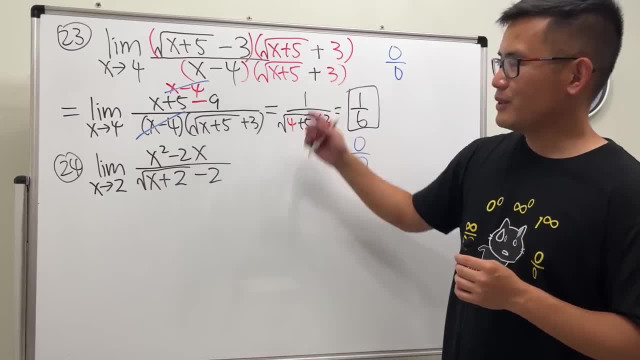 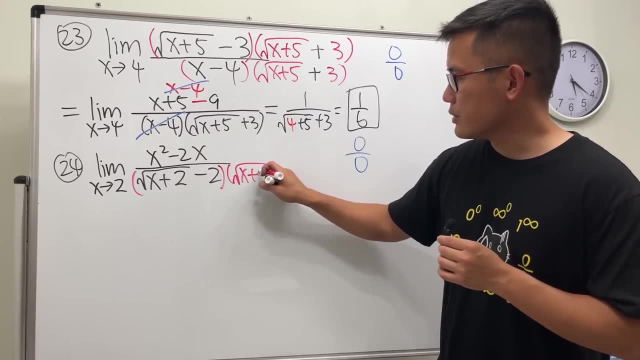 A 0 over 0 case. Don't worry, Conjugate again. Fix the square root part first. So I'm going to multiply the bottom by square root of X plus 2, and then plus right plus 2.. And then do the same. 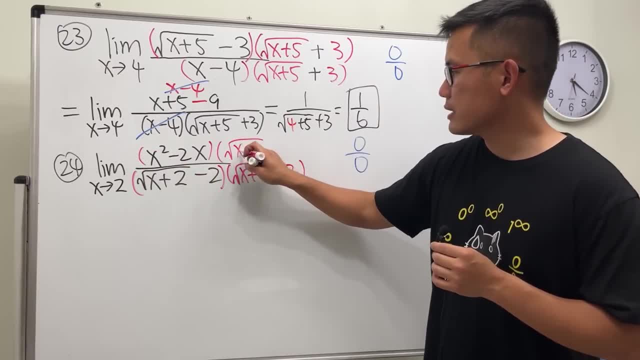 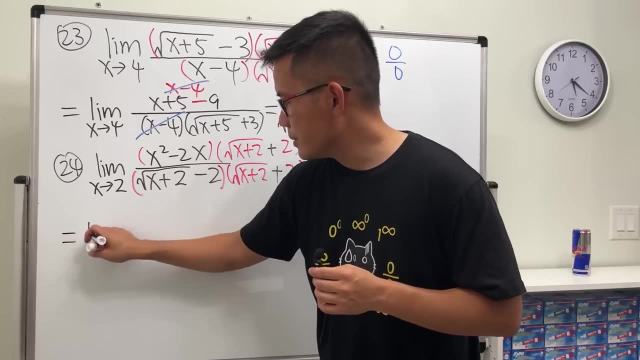 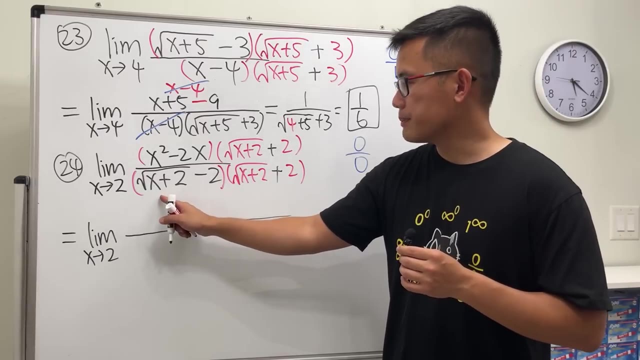 thing on the top Right here, square root of X plus 2 and then plus 2.. So let's fix the bottom first. This is going to be the limit as X approaching 2.. Just like what we said earlier, we square the first part, which is just going to be the X plus 2. 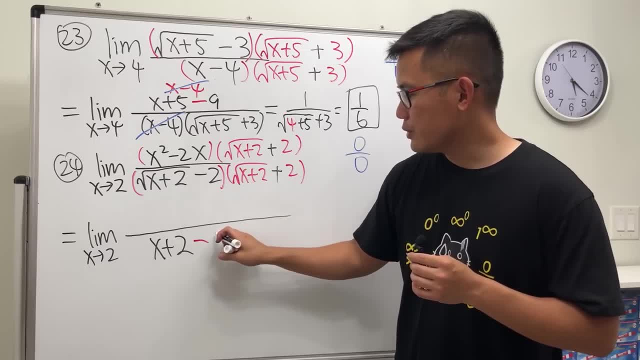 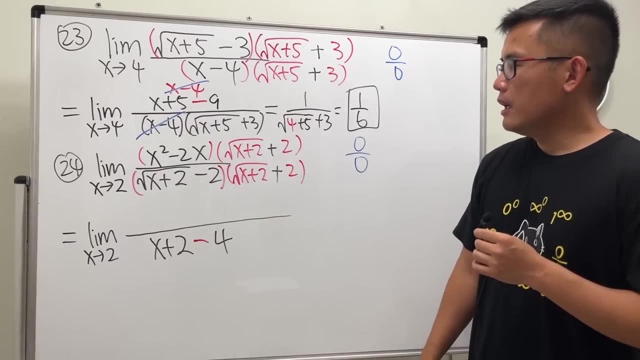 now, And then minus square root of the second, which is 2, squared, which is 4.. So that's a fast way to multiply all the conjugates On the top, though I'm not going to multiply the L Actually. 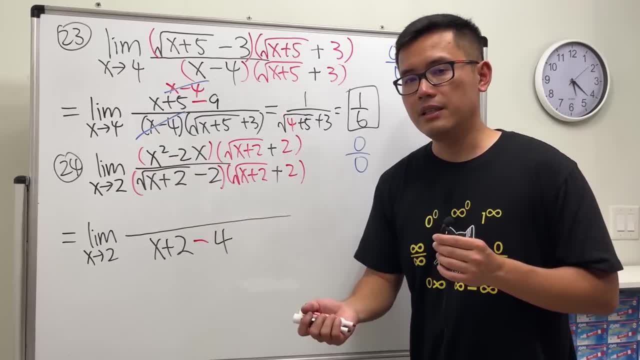 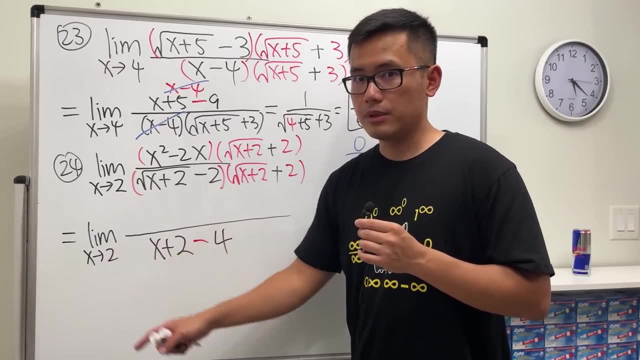 I'm going to factor this Because, as I said earlier, when we get a 0 over 0 situation, you're expecting to cancel out X minus 2, because X is approaching 2.. That's how we can end up with, that's how we can get rid of. 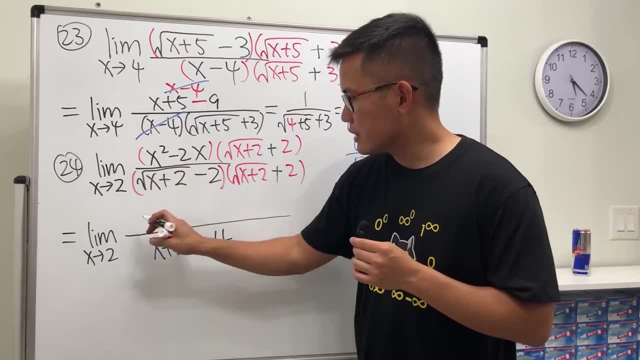 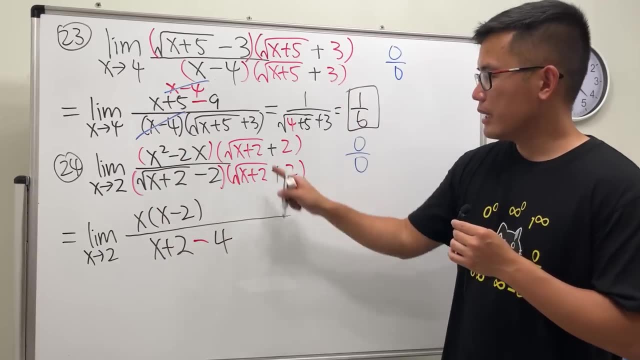 the 0 over 0.. Anyway, from here, I'm going to factor out an X, So keep that in black. So here we get X minus 2.. So this part is from there. This part, I'll keep it. I'll just write it in red. so 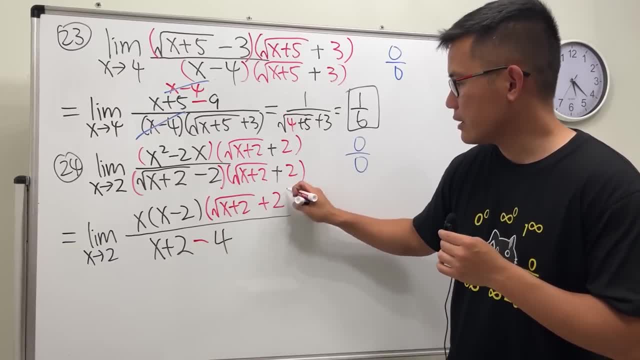 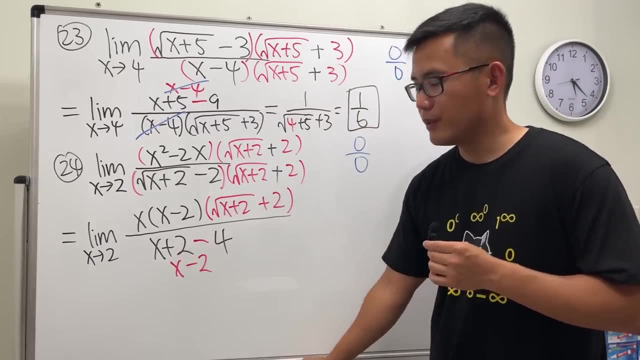 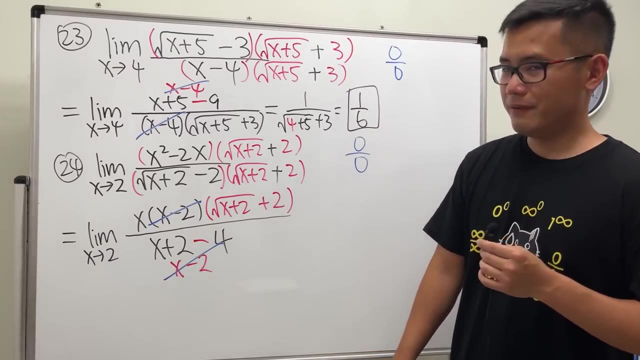 that you can see that this is the part that we had earlier. What's this? Yeah, this is just X minus 2, right? What can we do next? Yeah, ladies and gentlemen, X minus 2 and X minus 2, cancel, very much. 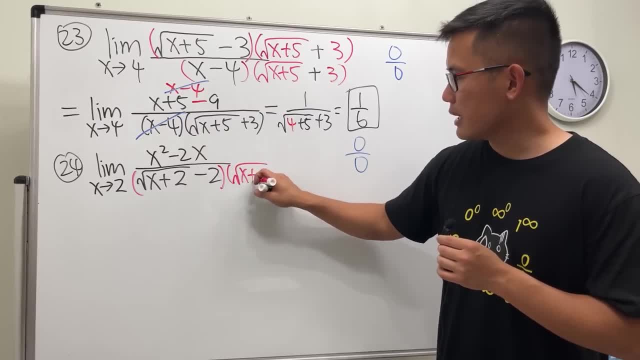 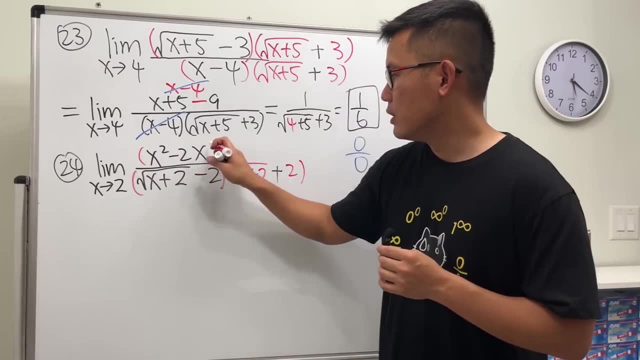 So I'm going to multiply the bottom by square root of x plus 2.. And then plus right, plus 2.. And then do the same thing on the top Right here: square root of x plus 2.. And then plus 2.. 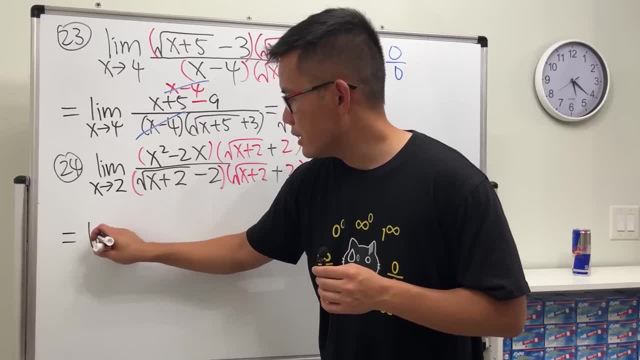 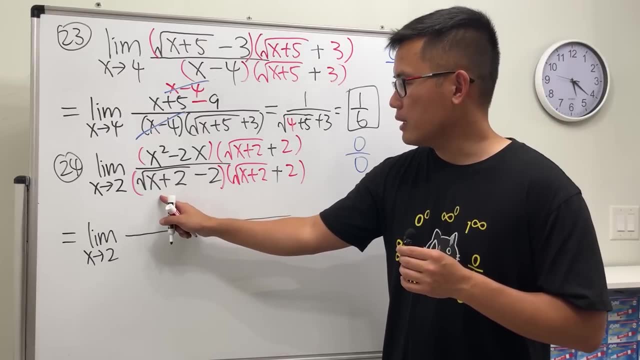 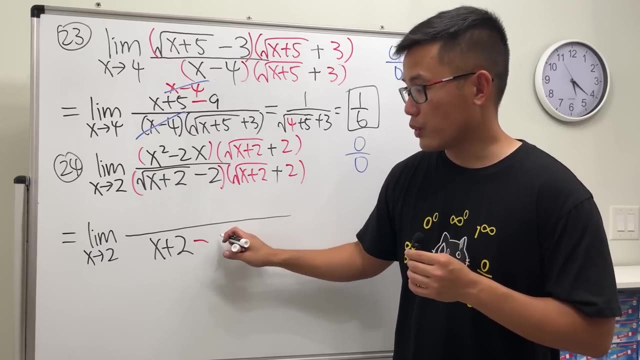 So let's fix the bottom first. This is going to be the limit as x approaching 2.. Just like what we said earlier, we square the first part, which is just going to be the x plus 2 now, And then minus square root of the second, which is 2 squared, which is 4.. 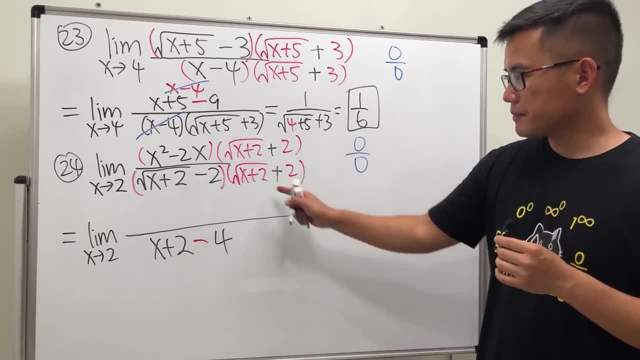 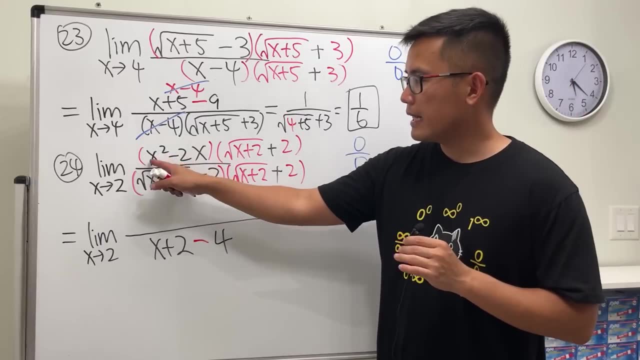 So that's the fast way to multiply all the counts you get On the top, though I'm not going to multiply the L. Actually, I'm going to factor this Because, as I said earlier, when we get a 0 over 0 situation, 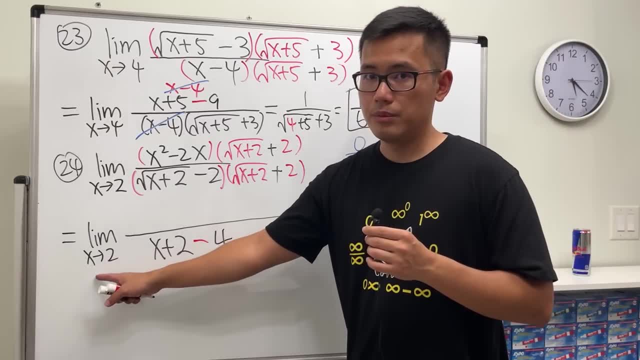 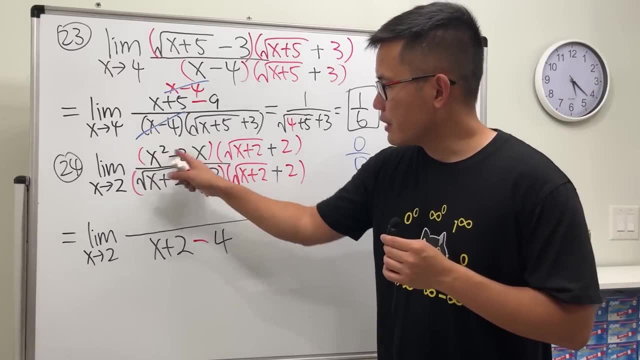 you're expecting to cancel out x minus 2, because x is approaching 2.. That's how we can end up with, that's how we can get rid of the 0 over 0.. Anyway, from here, I'm going to factor out an x. 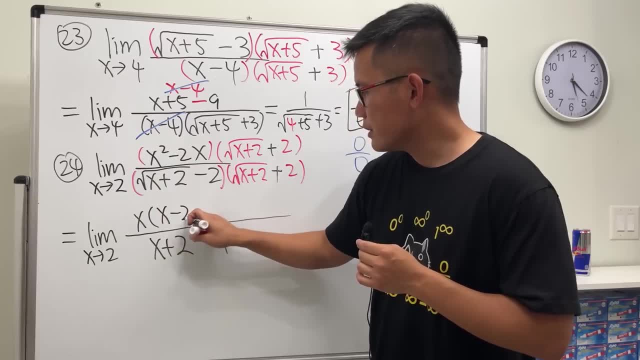 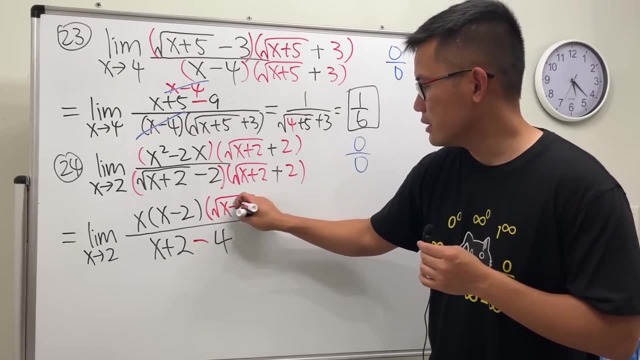 So keep that in black. So here we get x minus 2.. So this part is from there. This part, I'll keep it. I'll just write it in red so that you can see that this is the part that we had earlier. 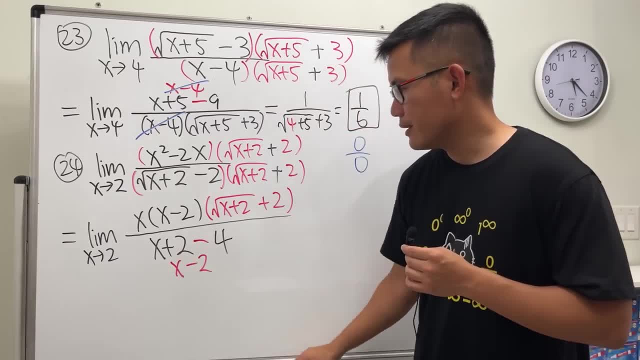 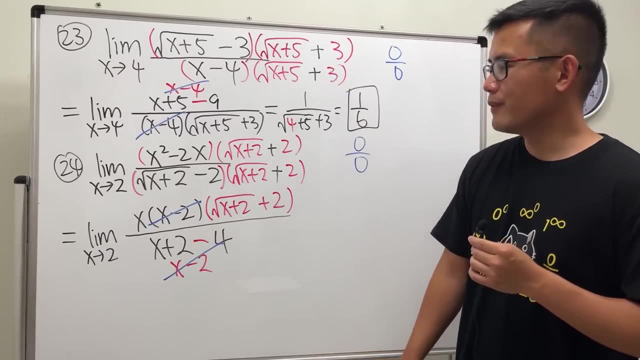 What's this? Yeah, This is just x minus 2, right. What can we do next? Yeah, Ladies and gentlemen, x minus 2 and x minus 2, cancel, very much, All right. So now we can just go ahead plugging 2 into here. 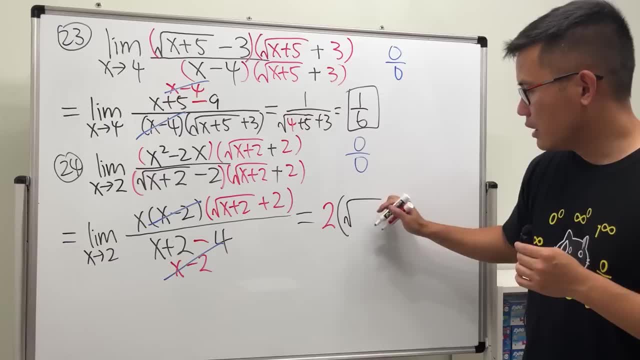 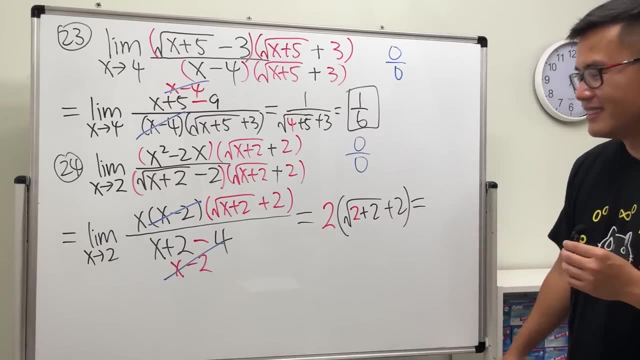 So we have a 2 here times square root of 2 plus 2 plus 2.. Who came up with this question? So many 2s? Yes, I did. Anyway, this is 2.. Plus 2 is 4, times 2, 8.. 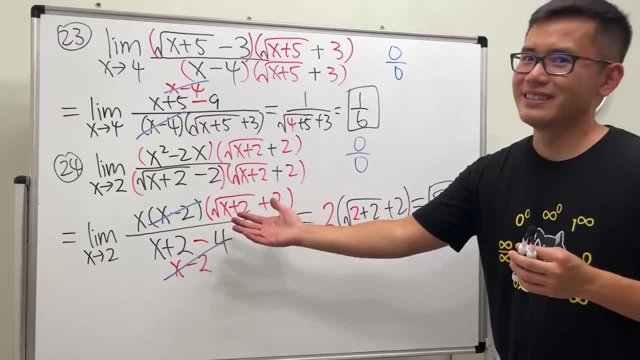 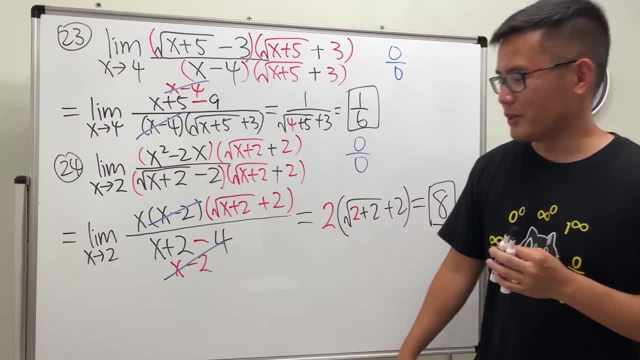 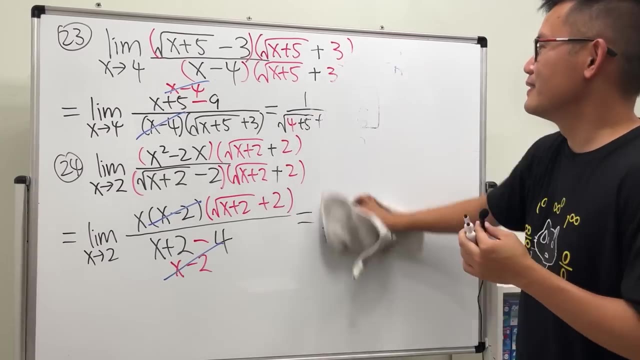 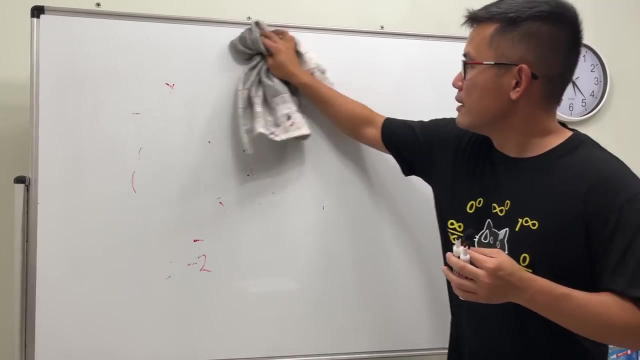 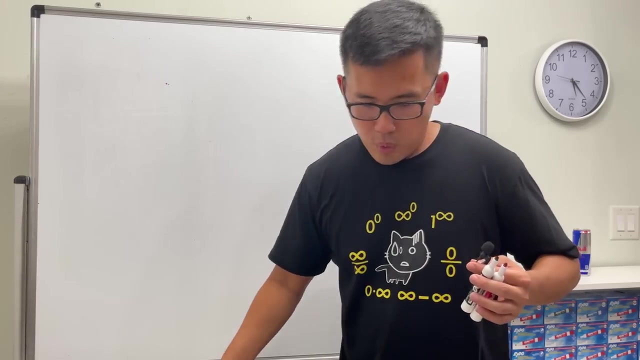 All right Done. So, oh look, I remember why I came up with this 8 and 24.. Rest in peace, Kobe Bryant. You think I didn't set this up? Of course I did. It's hot. 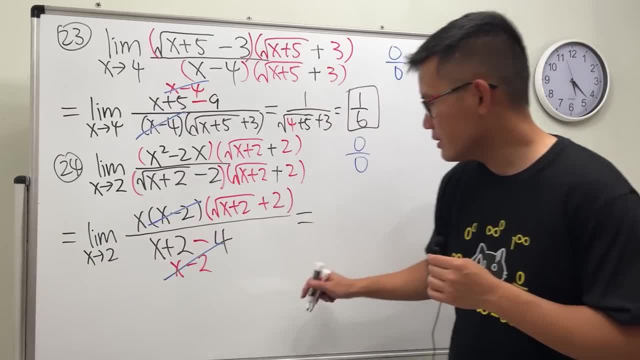 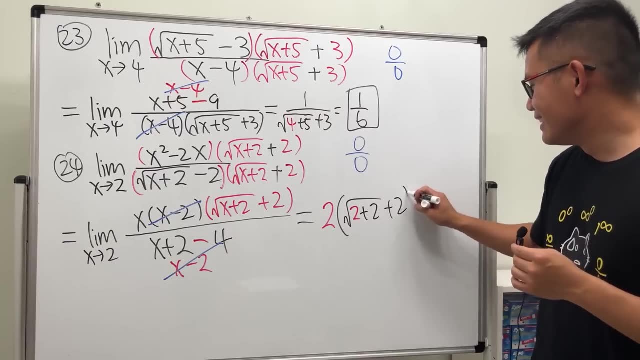 All right, so now we can just go ahead plugging 2 into here. So we have a 2 here times square root of 2 plus 2 plus 2.. Who came up with this question? So many twos? Yes, I did. Anyway, this is 2. 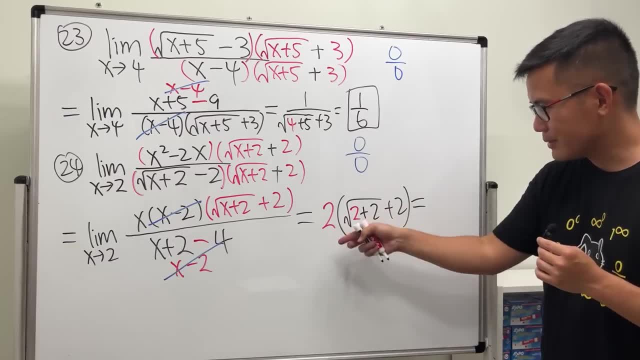 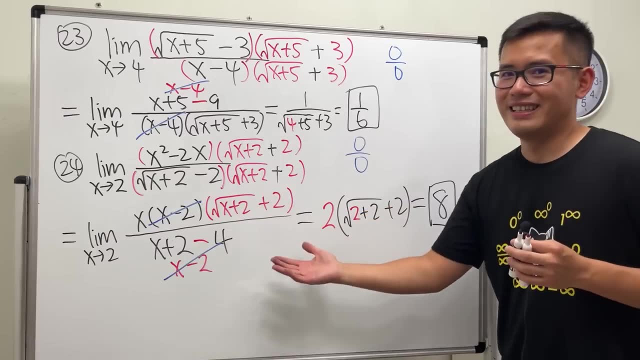 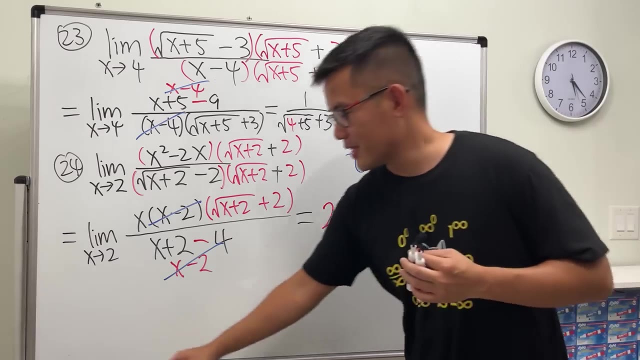 plus 2 is 4 times 2, 8.. All right, done. So oh look, I remember why I came up with this 8 and 24.. Rest in peace, Kobe Bryant, You think I didn't set this up? Of course I did. 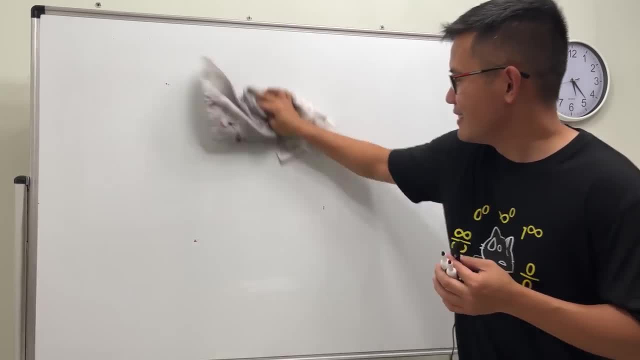 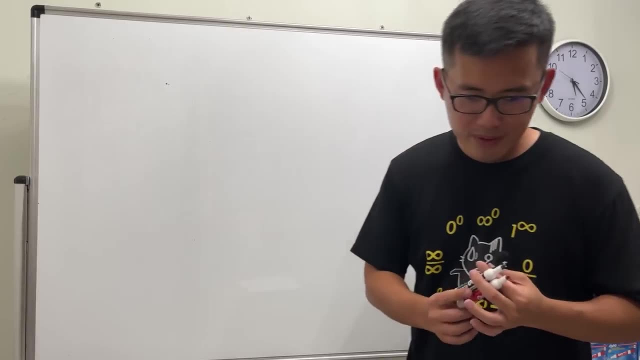 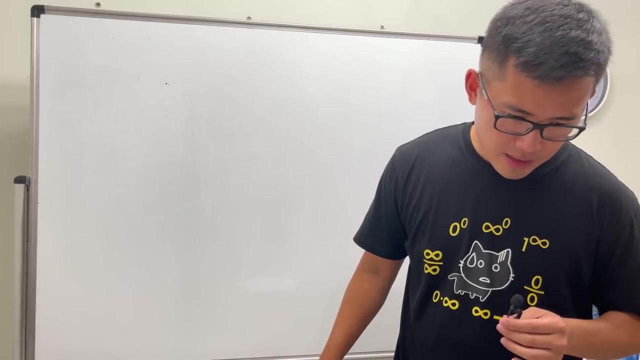 So I'm going to, I'm just going to, I'm going to. It's hot Anyway. Number 25.. Number 25.. Hey, you know what We're going to do. another limit. Hey, you know what We're going to do. another limit. 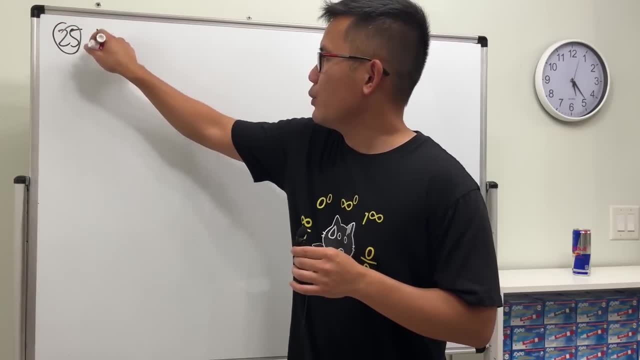 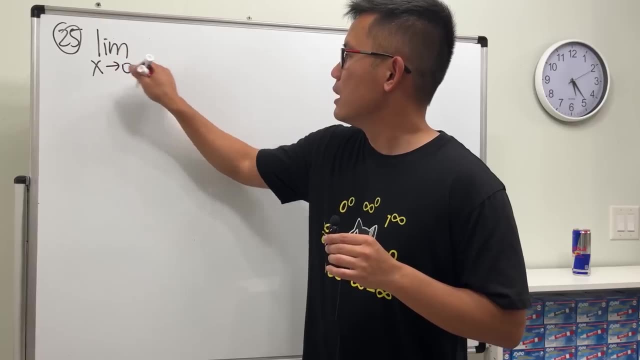 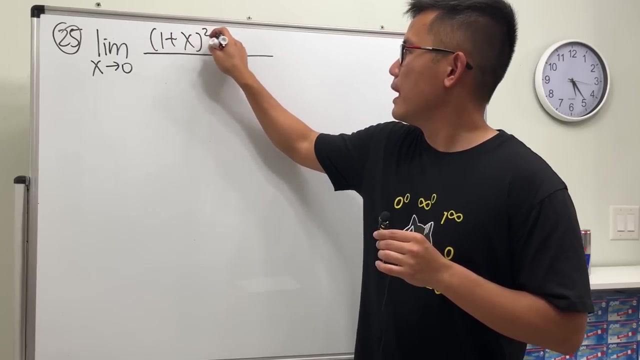 VSD limit as X approaching 0.. VSD limit as X approaching 0.. VSD limit as X approaching 0.. VSD- VSD: on the top we have 1 plus x squared minus 1, and on the bottom we have 1 plus x to the third power. 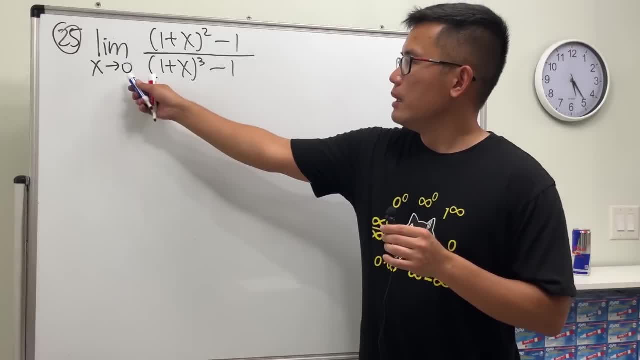 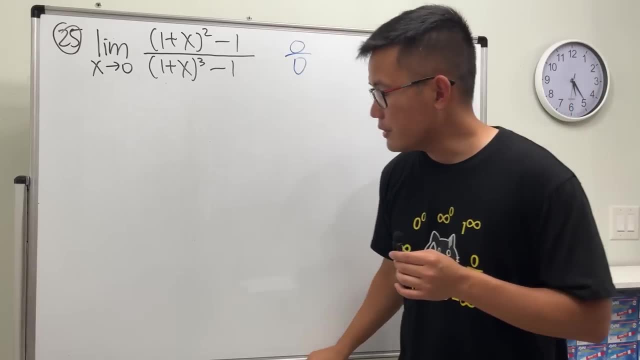 and then minus 1. yes, if you plug in 0, you get 1 minus 1 on top and likewise 1 minus 1 on the bottom, so this is a very clear 0 for 0 situation. do more work. what do we do, though? well, 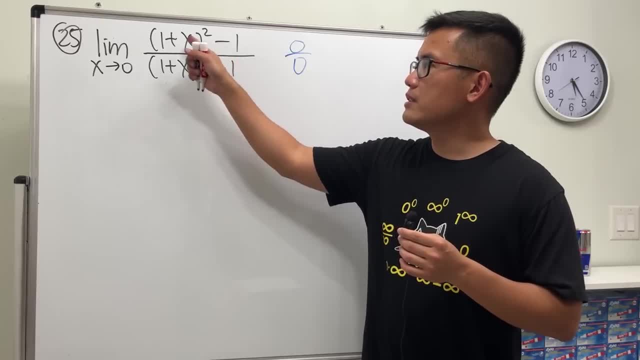 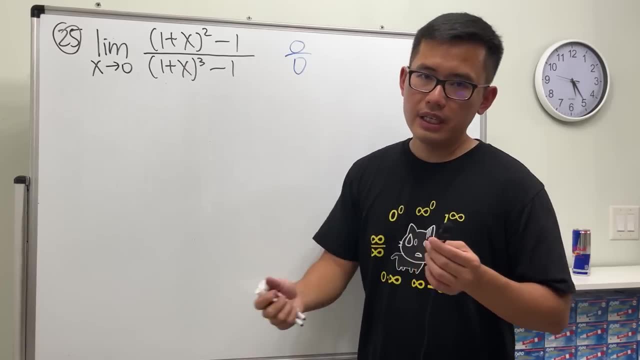 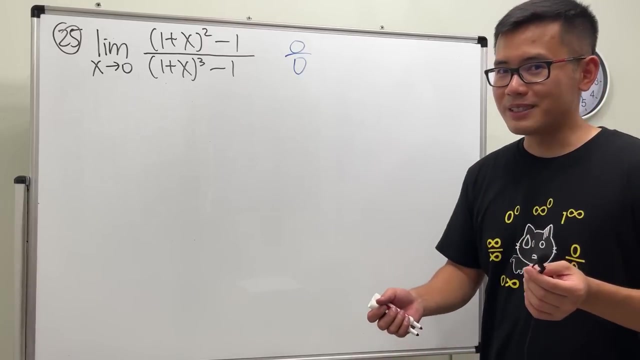 on the top, technically it's a difference of two squares. so if you are a fan of factoring, be my guest. on the bottom is a difference of two cubes. again, if you are a fan of factoring, be my guest. you can also multiply it out. so if you are a fan of multiplying things out, 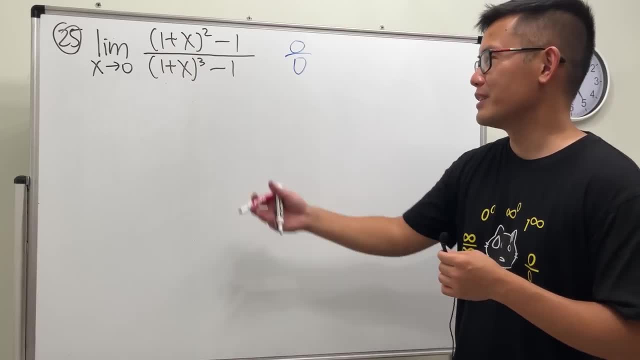 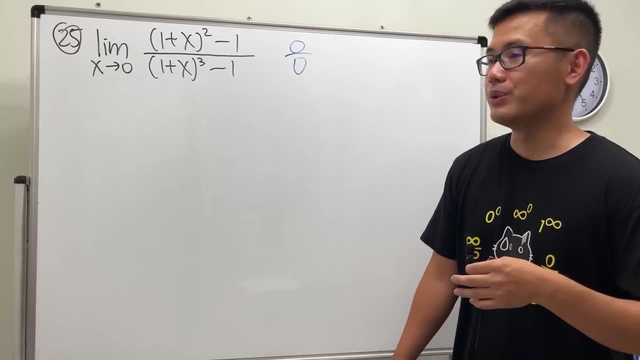 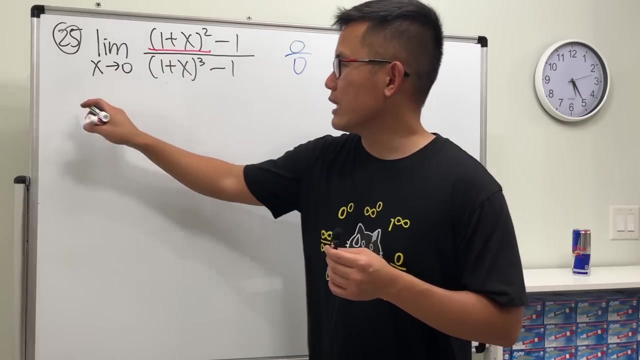 the binomial part be my guest. likewise the bottom be my guest. so i'm going to do it the more natural way that i think most of the students will do, which is actually just multiply the out. usually multiplying out is more, not necessarily natural, not necessarily easier, but 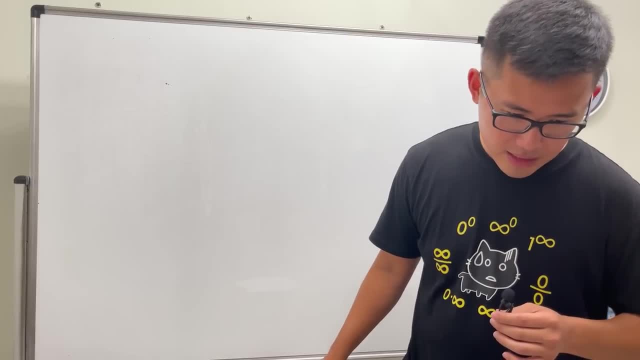 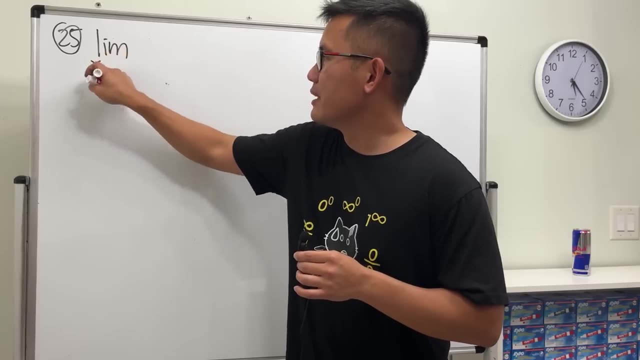 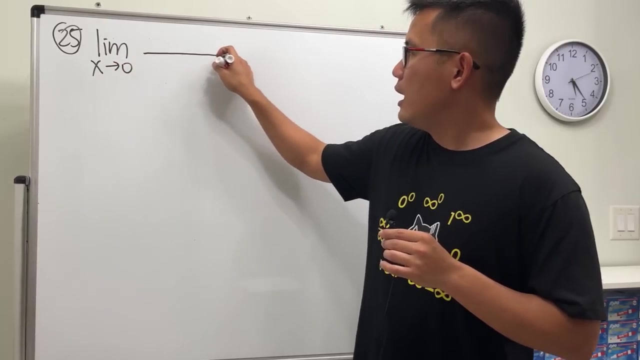 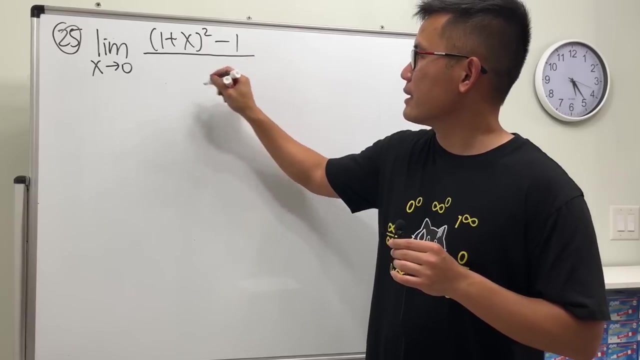 Anyway, Number 25.. Hey, you know what We're going to do. another limit, Obviously limit as x approaching 0. So on the top we have 1 plus x squared minus 1, and on the bottom we have 1 plus x to the third power and then minus 1.. 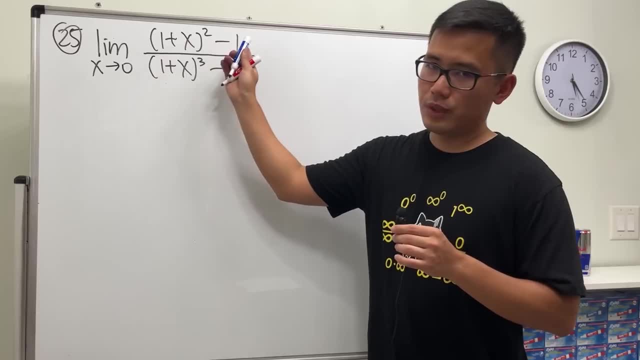 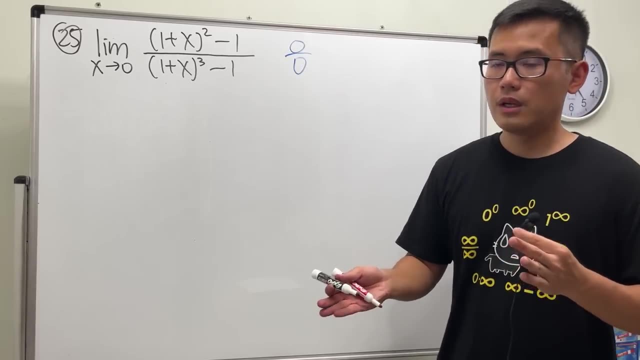 Yes, if you plug in 0, you get 1 minus 1 on top and likewise 1 minus 1 on the bottom, So this is a very clear 0 for 0 situation. Do more work. What do we do, though? 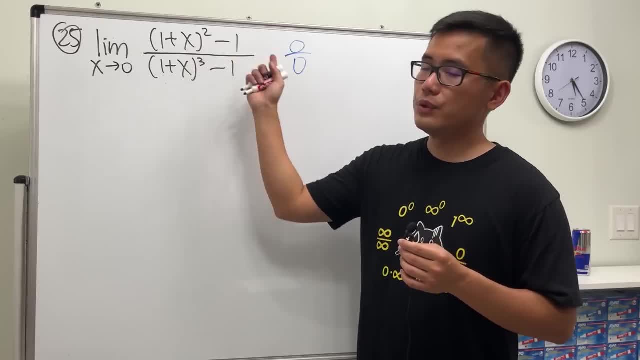 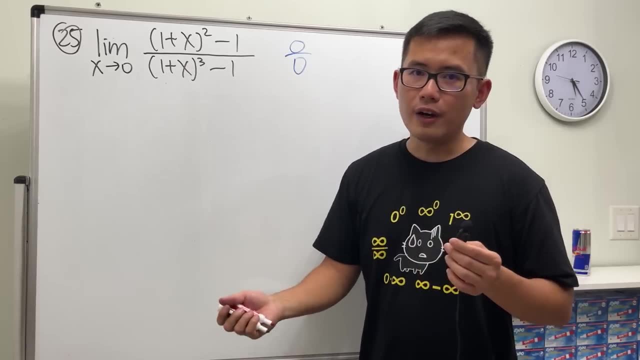 Well, on the top, technically it's a difference of 2 squared. So If you are a fan of factoring, be my guest. On the bottom, it's a difference of 2 cubes. Again, if you are a fan of factoring, be my guest. 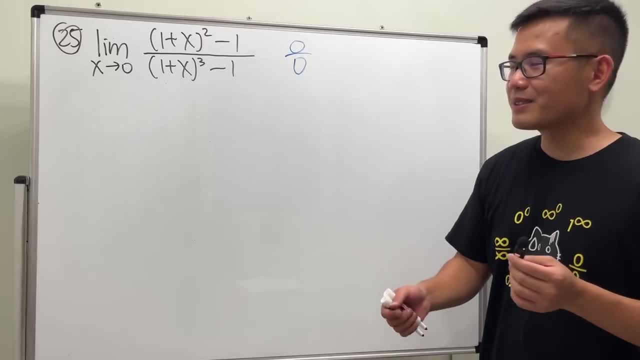 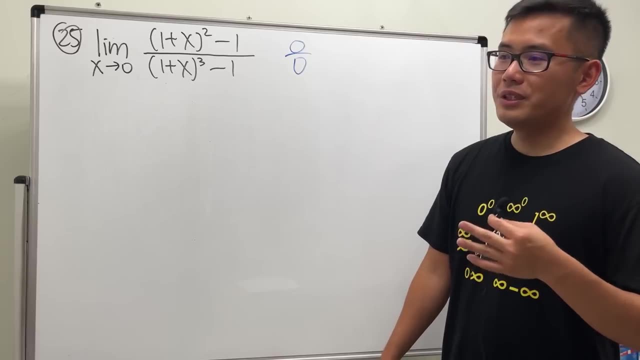 You can also multiply the out. So if you are a fan of multiplying things out, the binomial part be my guest. Likewise, the bottom be my guest. So I'm going to do it the more natural way that I think most of the students will do, which is actually just multiply the out. 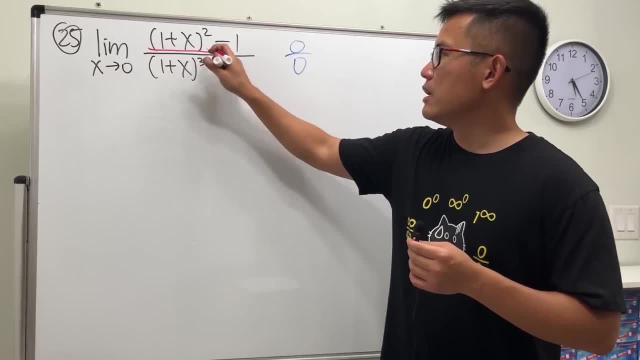 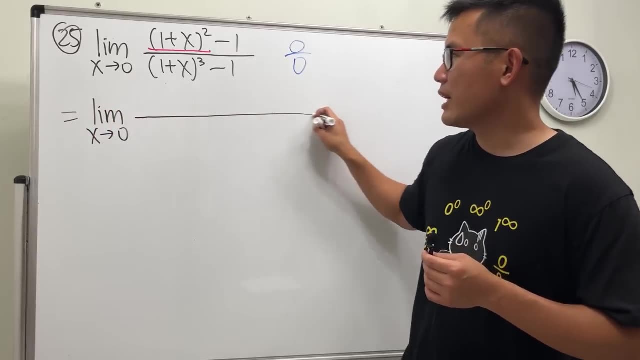 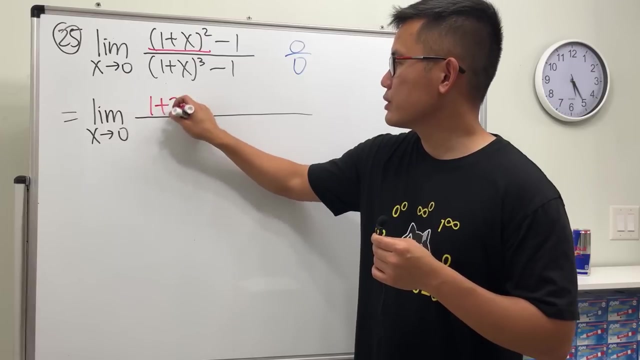 Usually multiplying out is more, Not necessarily natural, not necessarily easier, but more direct. I would say: So yeah, 1 plus x squared. just write 1 plus x times 1 plus x. multiply the out, we get 1 plus 2x plus x squared. 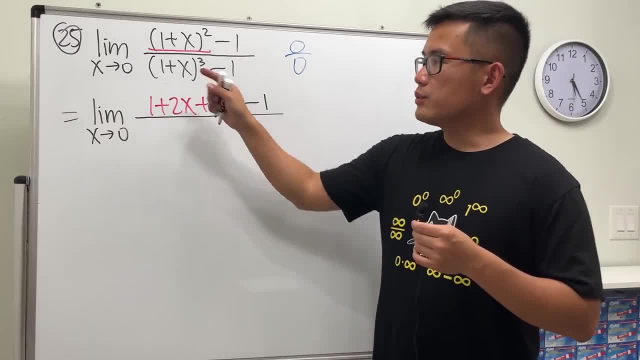 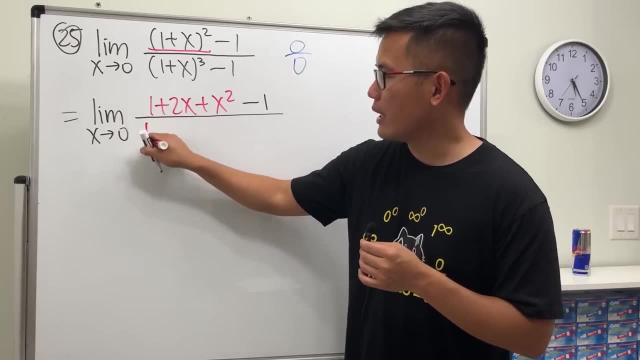 And then we have that minus 1.. This right here, just to impress you guys. I'll show you guys what the answer is. What we do is we do 1 to the third power, which is 1, plus 3 times 1 to the second power, which is 3.. 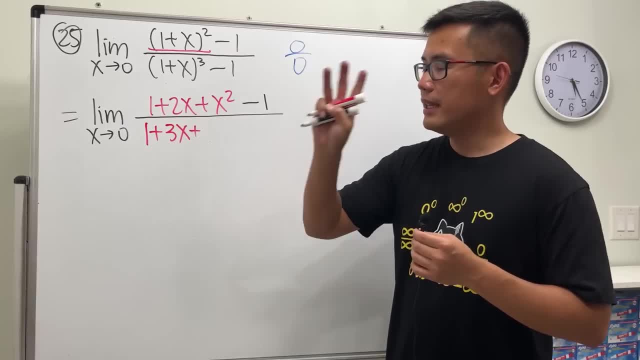 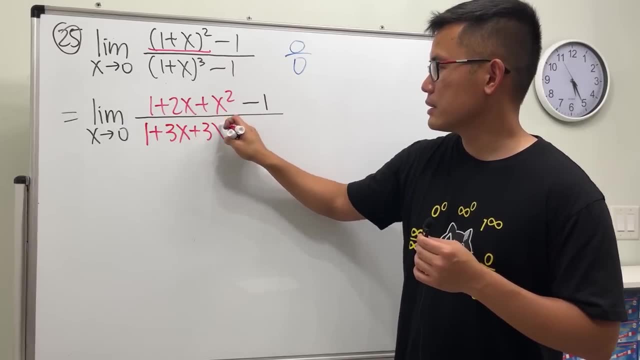 And then times x to the first power Next, and then use 3 again as a coefficient: 3 times 1 to the first power, which is still 3, times x to the second power And, lastly, x to the third power. 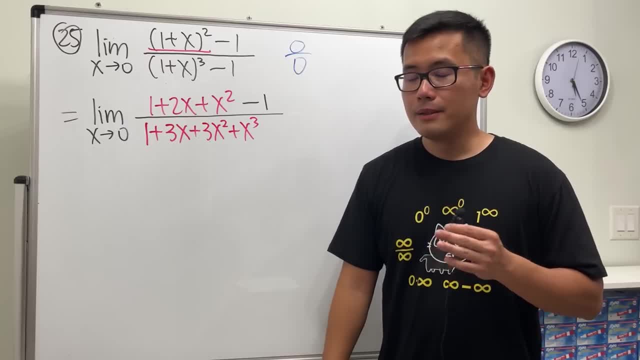 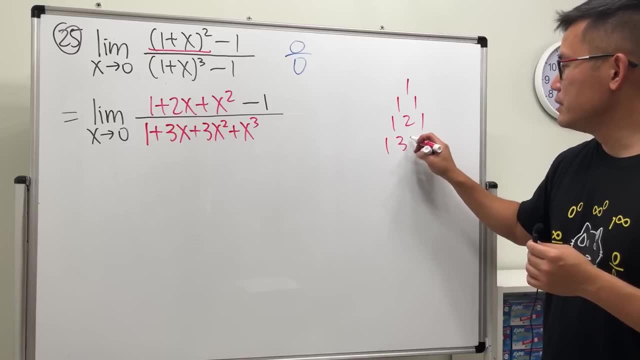 So that's the Pascal's triangle or the binomial coefficient. So 1, 1, 1.. And then 1, 2, 1.. 1, 3, 3. 1.. That's why I used 3 and 3 earlier for these two coefficients. 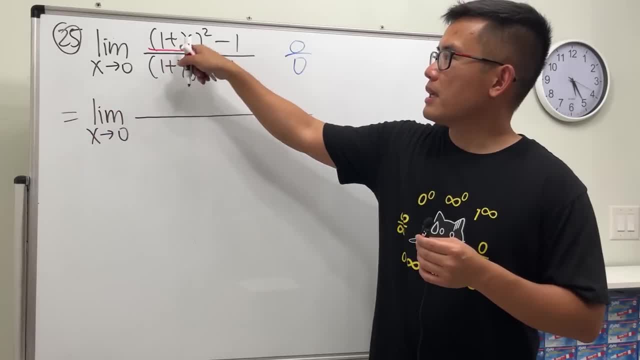 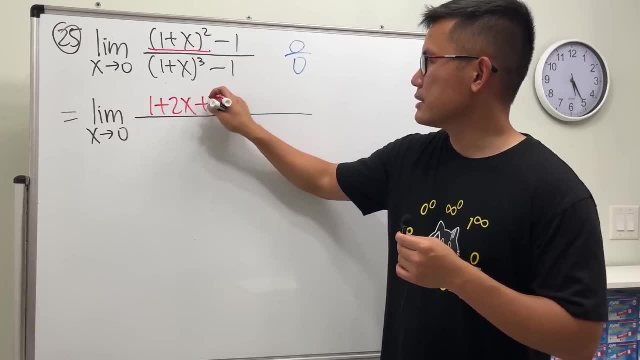 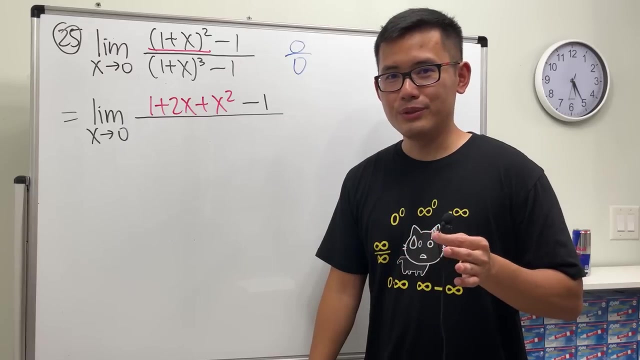 more direct. i would say: so yeah, 1 plus x squared. just write 1 plus x times 1 plus x, multiply the out. we get 1 plus 2x plus x squared, and then we have that minus 1.. this right here, just to impress you guys. i'll show you guys what the answer is. what we do is we do 1 to the third. 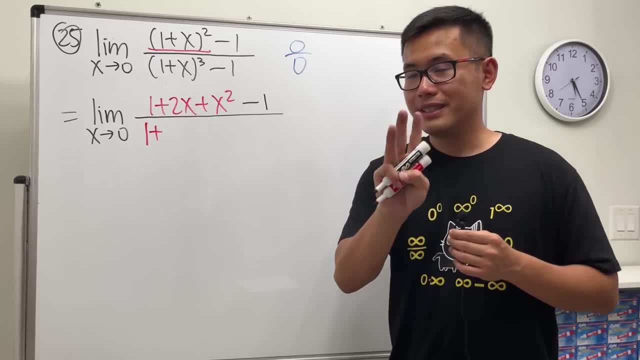 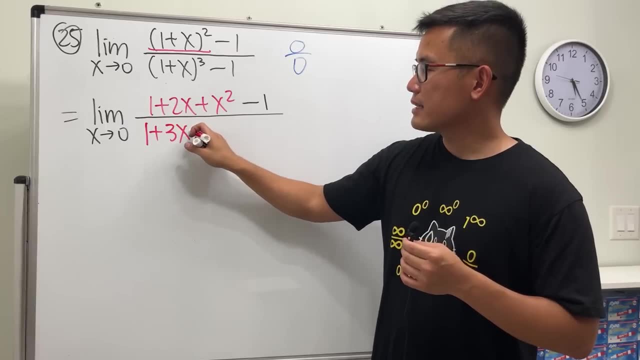 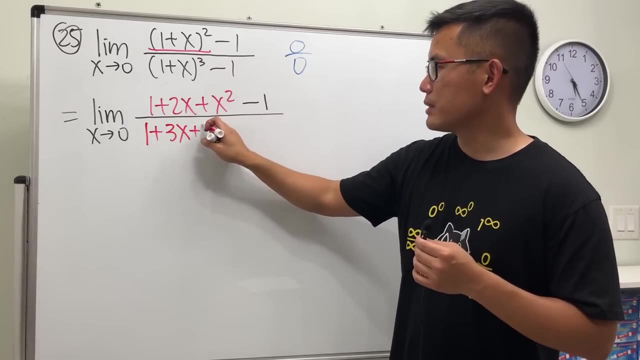 power, which is 1 plus 3 times 1, to the second power, which is 3, then times x to the first power next, and then use 3, again as a coefficient, 3 times one to the first power, which is still 3 times x to the second power. 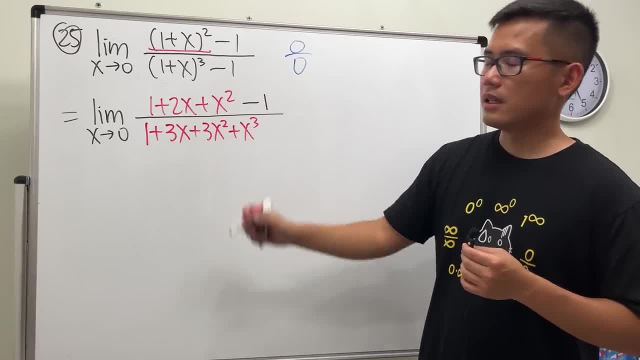 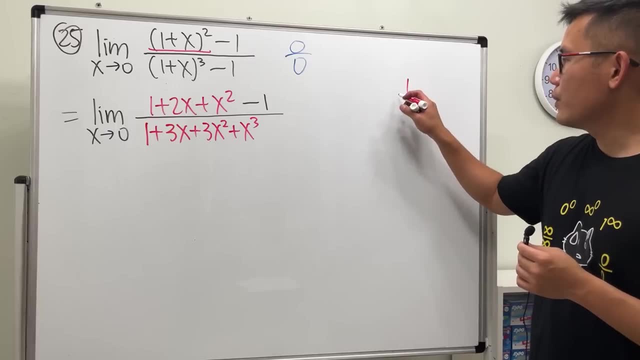 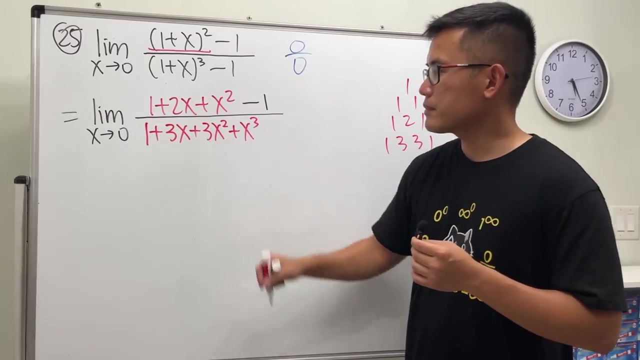 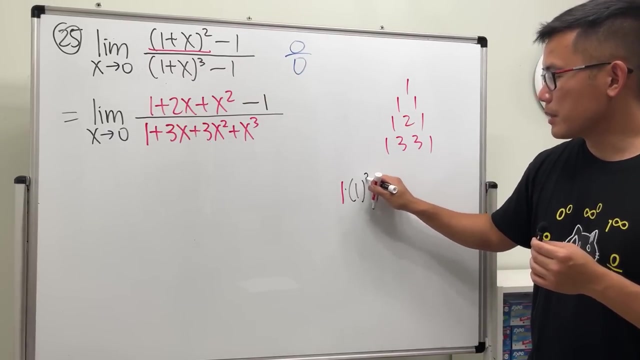 and lastly, x to a third power. so that's the pascal's triangle or the binomial coefficient. so, and then one, two, one, one, three, three, one. that's why i used three and three earlier for these two coefficients, and when i did this, technically i was doing one times one to the third power. 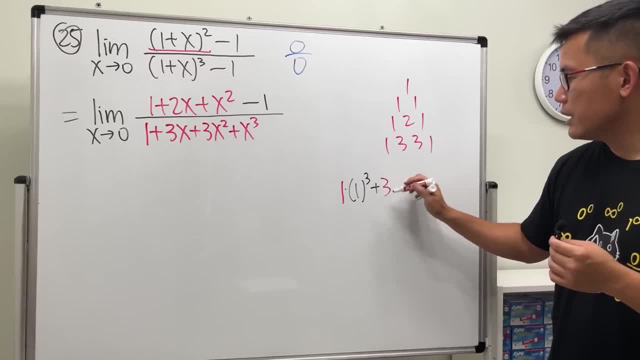 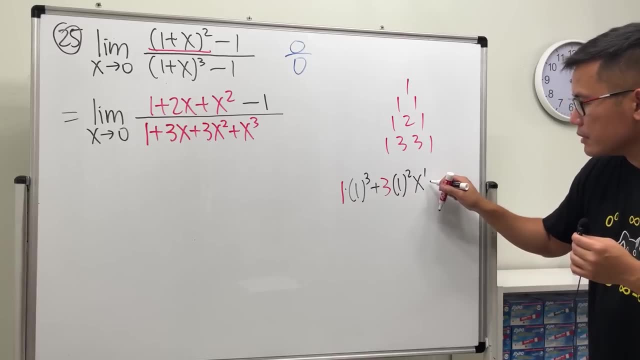 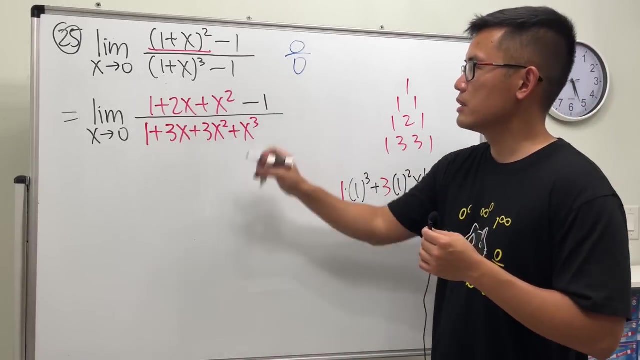 and then plus three times one to the second power. the power goes down and then the x power goes up, and then plus the next coefficient. so it's one first power, x square, and lastly plus one and then x to the third power. so that's how i did it pretty much, and then minus one, so you can take. 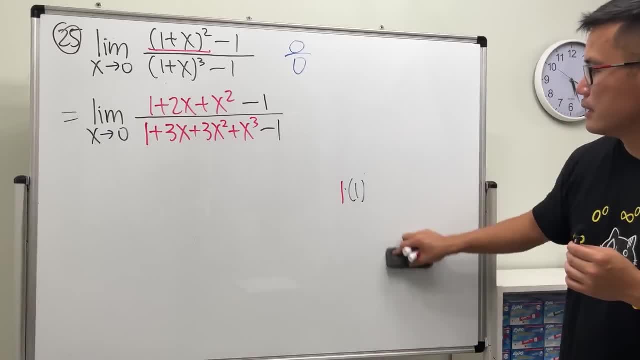 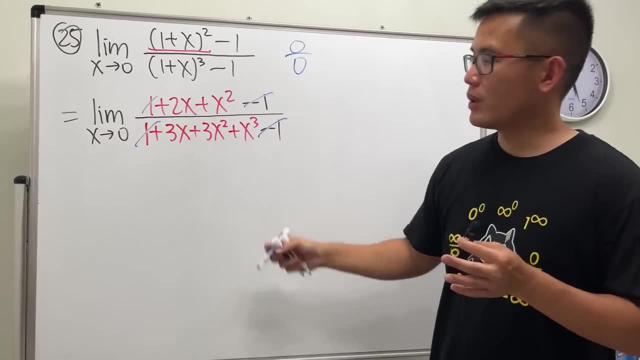 a look, all right, this is not so bad. you see, the one minus one, one minus one, pretty good. you see the one minus one, one minus one, pretty good. you see the one minus one, one minus one, pretty good. and then the beauty is that we can actually just factor out an x, and i think, for this one, let me 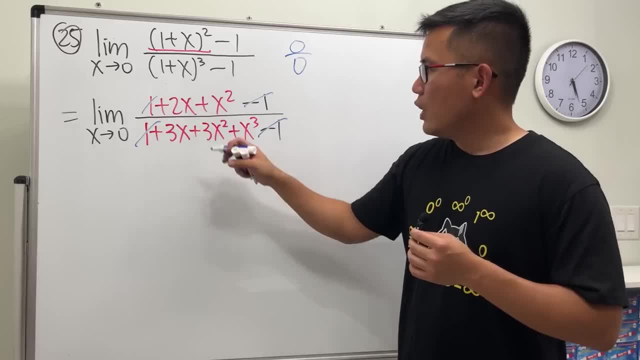 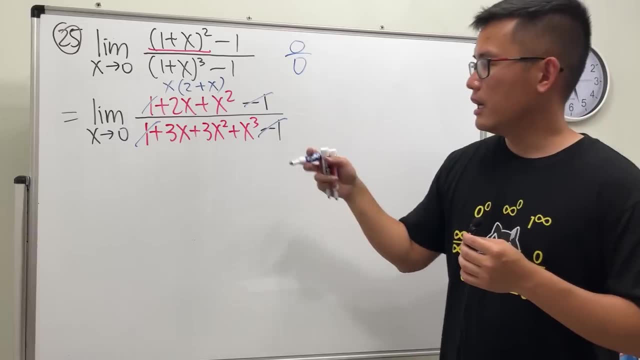 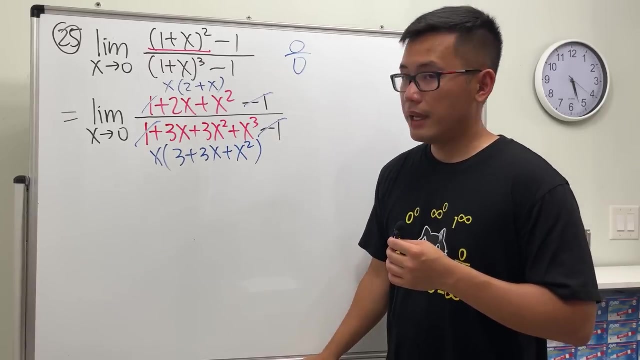 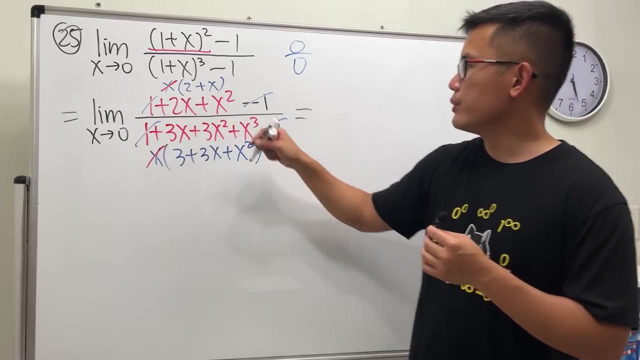 just yeah, let me just write it down right here. so let's see, when we factor on x, on the top, we get two plus x. yes, on the bottom, when we factor on x, we get three plus three, x plus x square, and then the x and x cancel, so finally we can put zero into. 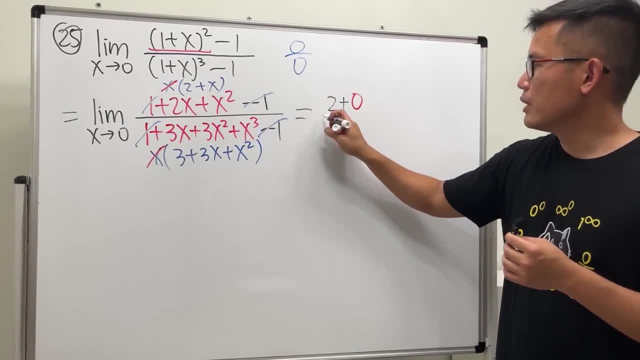 and then the x and x cancel, so finally we can put zero into and then the x and x cancel, so finally we can put zero into the. the x there, so two plus zero over zero into here. the x there, so two plus zero over zero into here. 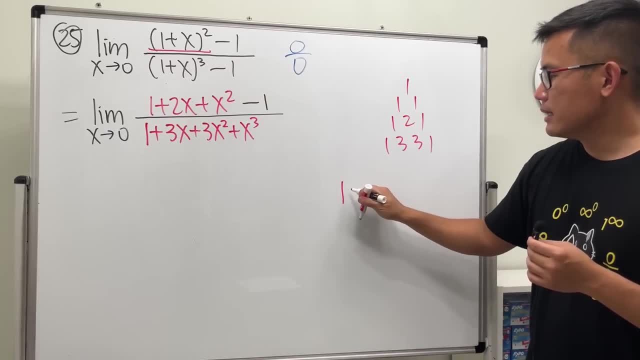 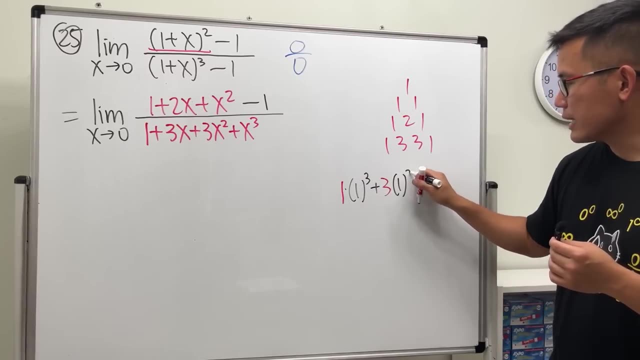 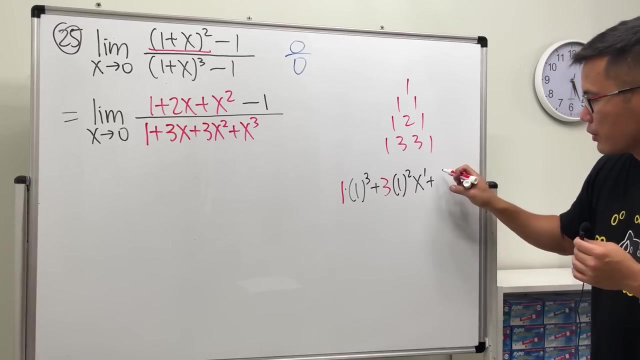 And when I did this, technically I was doing 1 times 1 to the third power And then plus 3 times 1 to the second power. The power goes down And then the x power goes up, And then plus the next coefficient. 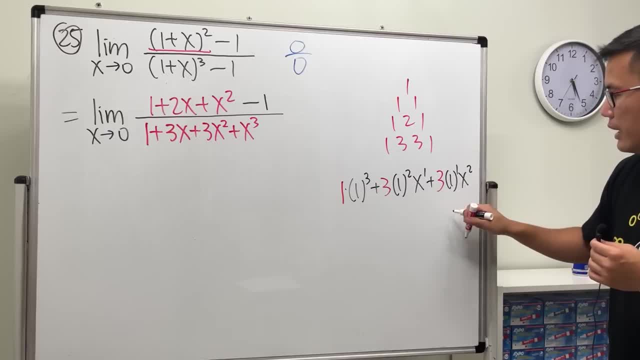 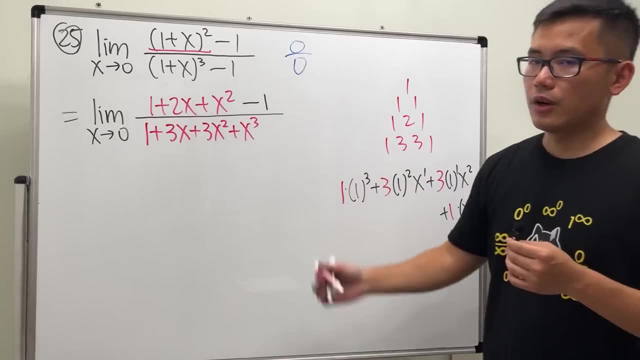 So it's 1, first power, x squared, And lastly plus 1.. And then And then x to the third power. So that's how I did it pretty much, And then minus 1.. So you can take a look. 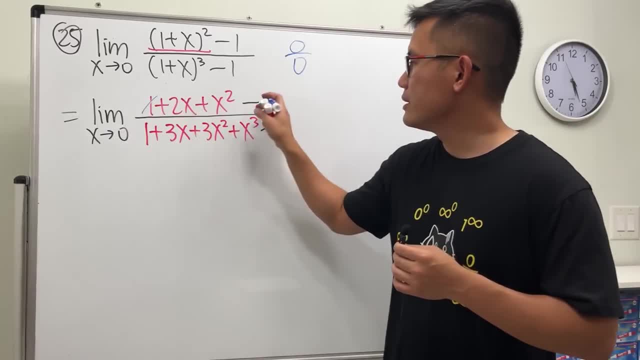 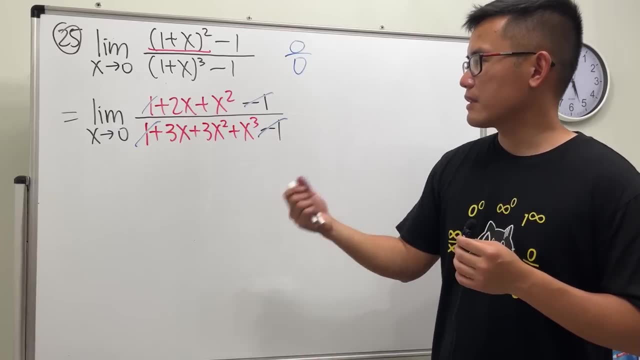 All right, This is not so bad. You see, the 1, minus 1, 1, minus 1.. Pretty good. And then the beauty is that we can actually just factor out an x, And I think, for this one, let me just, yeah, let me just write it down right here: 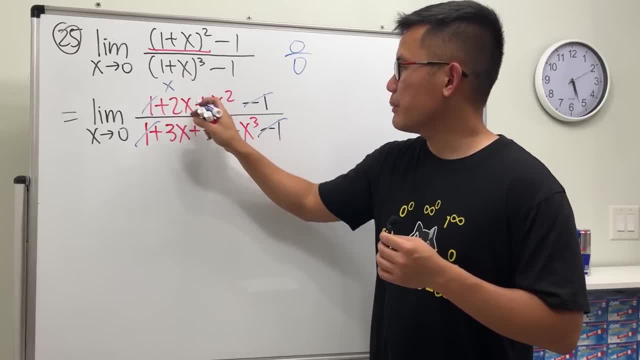 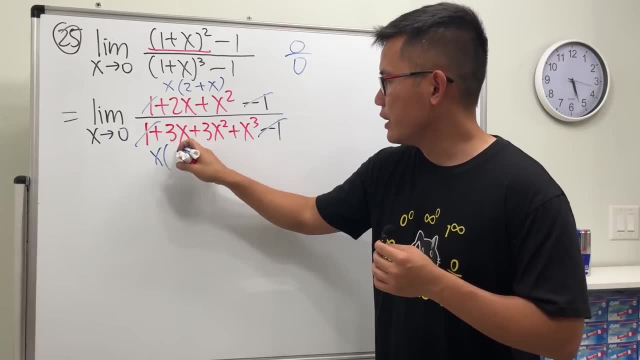 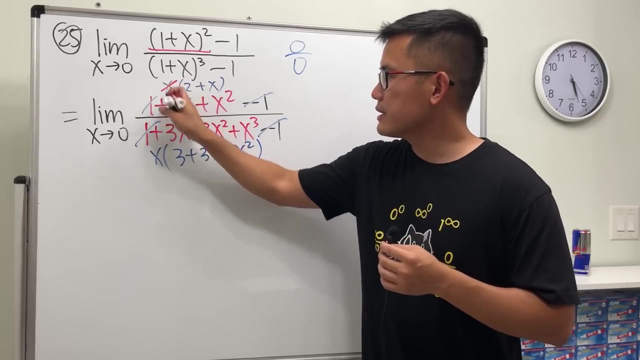 So let's see: When we factor out an x, On the top, we get 2 plus x, Yes. On the bottom, when we factor out an x, we get 3 plus 3x plus x squared, And then the x and x cancel. 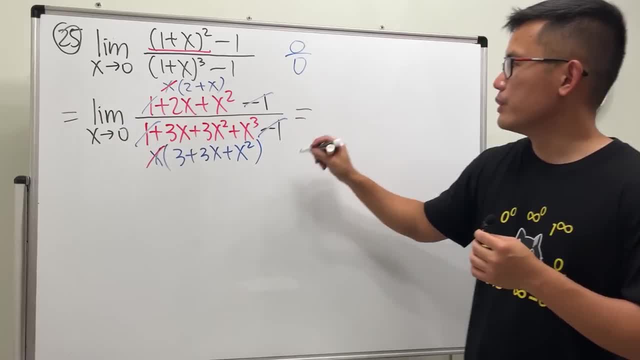 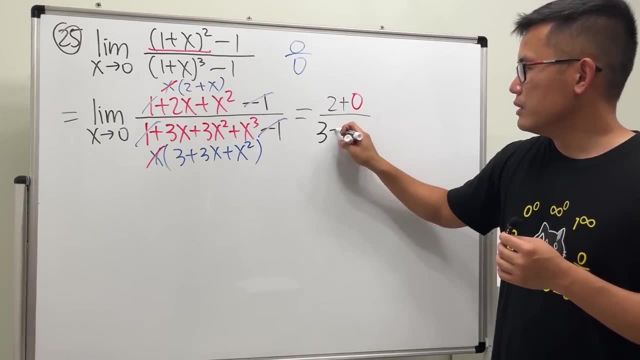 So finally we can put 0 into the x there. So 2 plus 0 over 0 into here. It's just 2 over 3, right, Because this right here will be 0. So yeah, So the final answer is just 2 over 3.. 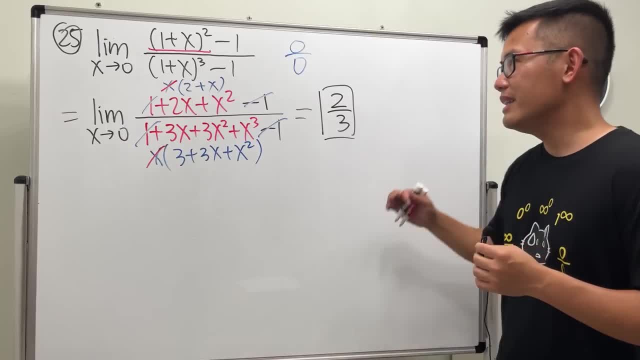 Yeah, All the x's are 0.. So just 2 over 3.. And then we are done. Yeah, So this is for that. And then, yeah, As I said this right here, I think it's more natural. 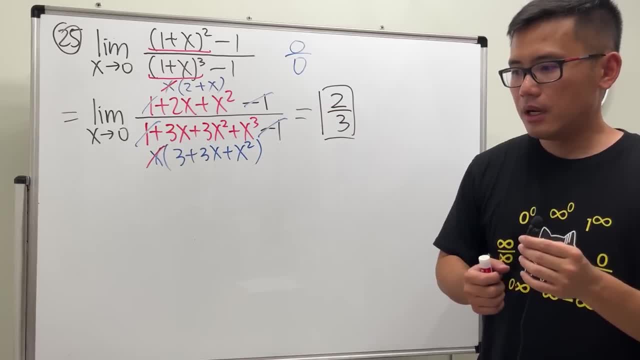 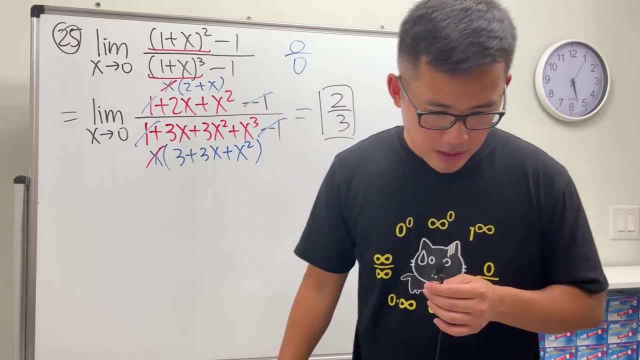 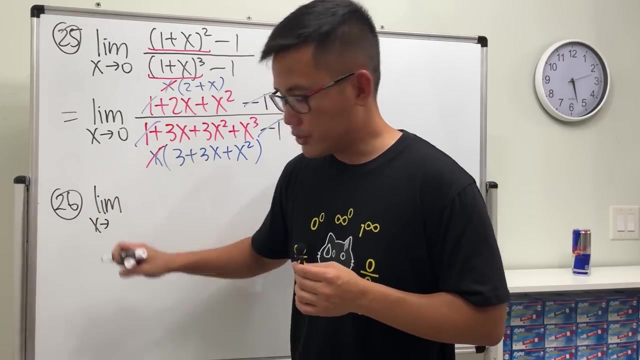 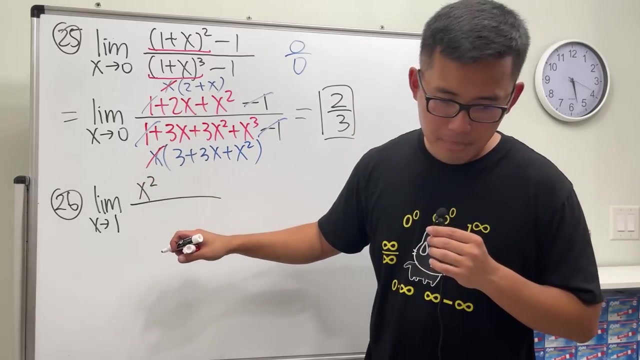 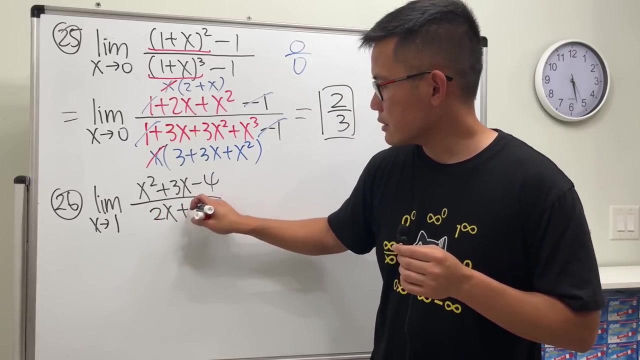 So if you do the factoring, you might be studying more this art. All right, Anyway, number 26.. Limit x approaching, we have 1x squared plus 3x minus 4 over 2x plus 10.. Okay, 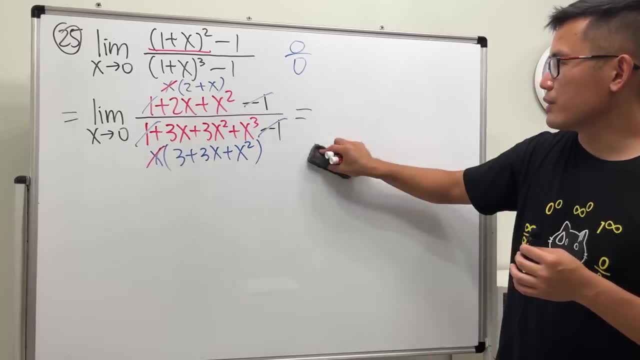 the x there. so two plus zero over zero into here. it's just two over three. right, because this it's just two over three. right, because this it's just two over three. right, because this right here will be zero. so right here will be zero, so right here will be zero. so yeah, so the final answer is just two over. 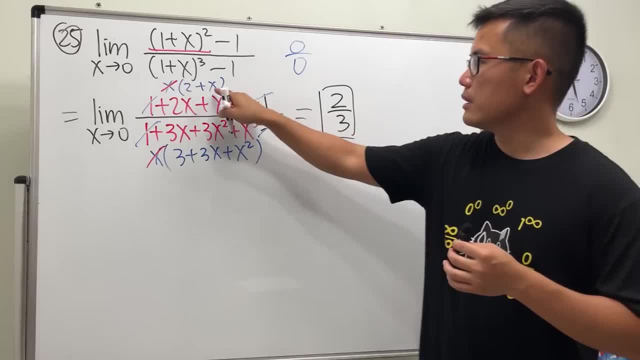 yeah, so the final answer is just two over yeah, so the final answer is just two over three, three, three. yeah, all the x's are zero, so just two. yeah, all the x's are zero, so just two. yeah, all the x's are zero. so just two over three. and then we are done. 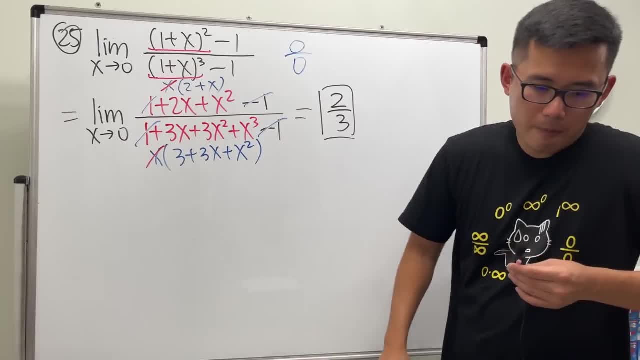 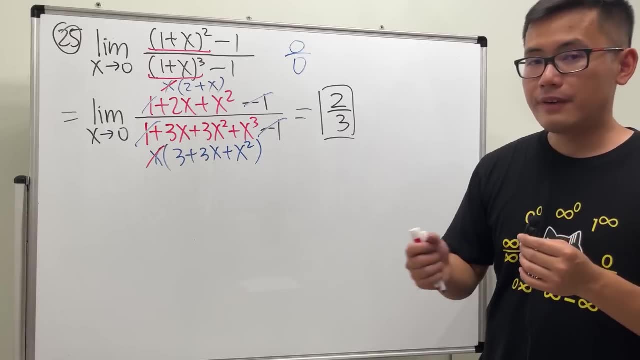 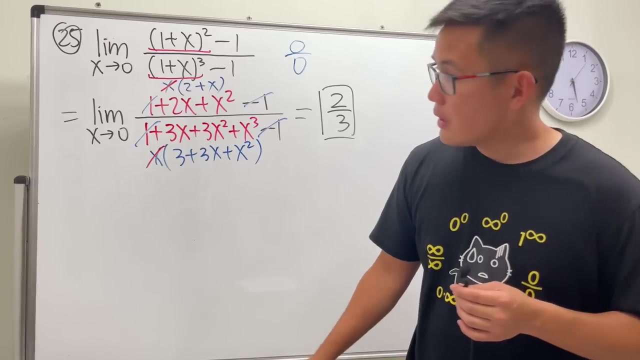 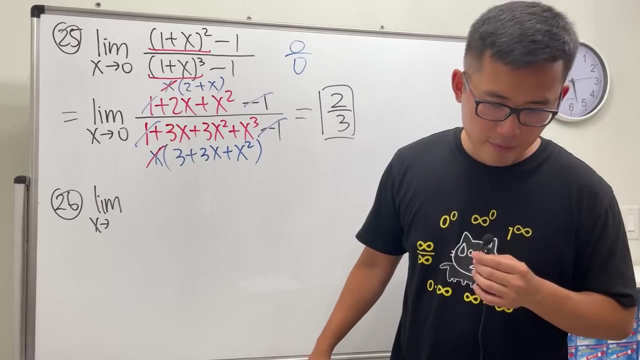 over three, and then we are done. yeah, so this is for that, and then, yeah, as i said this right here, i think it's more natural if you do the um factoring, it might be slightly more bizarre. all right, anyway, number 26: limit x approaching. we have one. 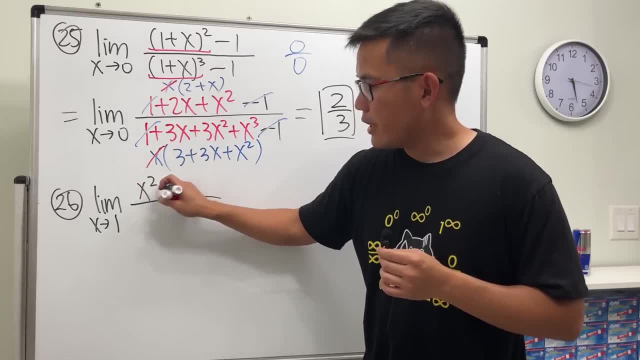 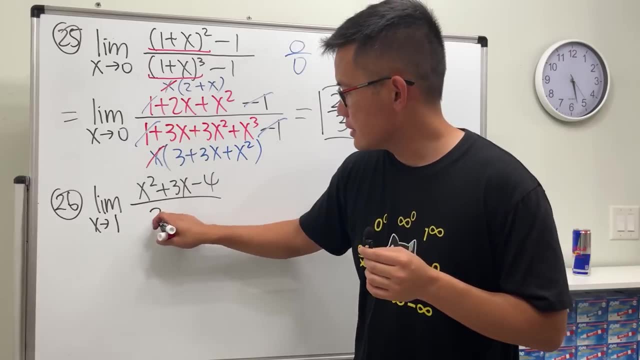 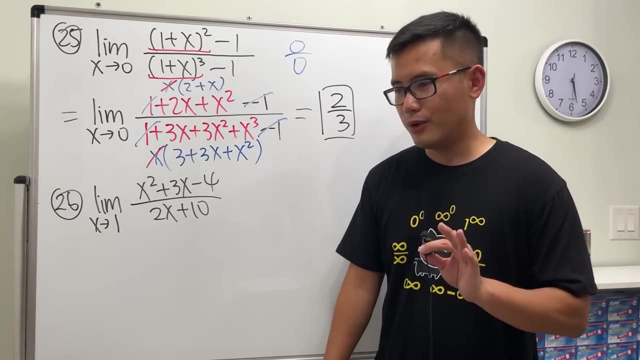 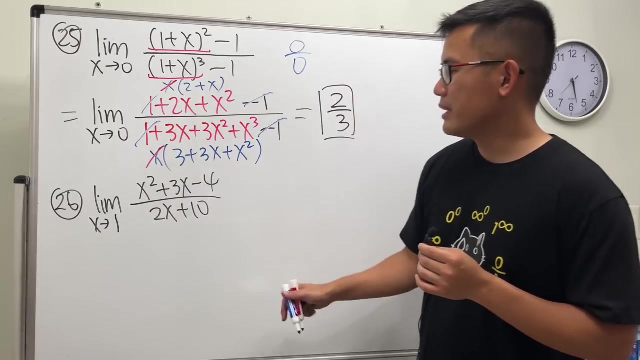 x squared plus 3x minus 4 over 2x plus 10.. okay, go ahead and factor and try to cancel. no, no, no, why again have the good habit? put the 1 into here. let's see what we get. so we get 1. 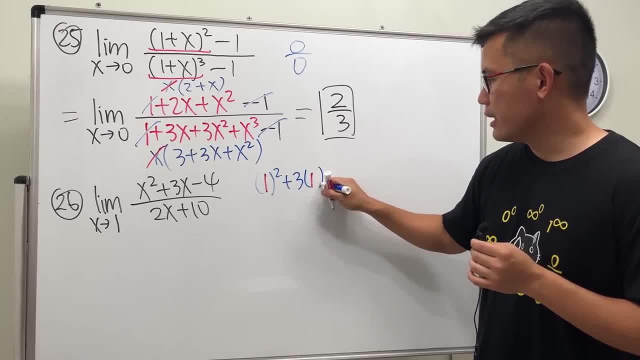 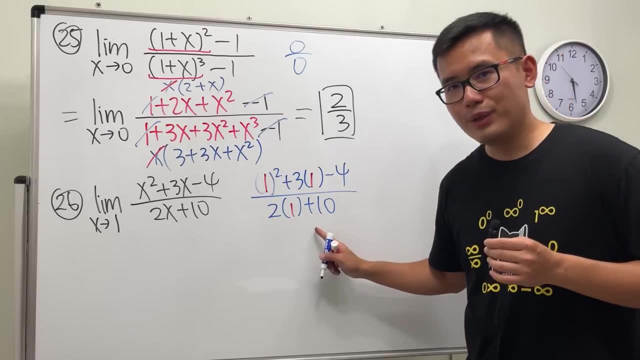 squared plus 3 times 1, 1, and then minus 4, over 2 times 1, and then plus 10.. Do we get 0 on the bottom? No, we don't. huh, It's the 12 on the bottom. 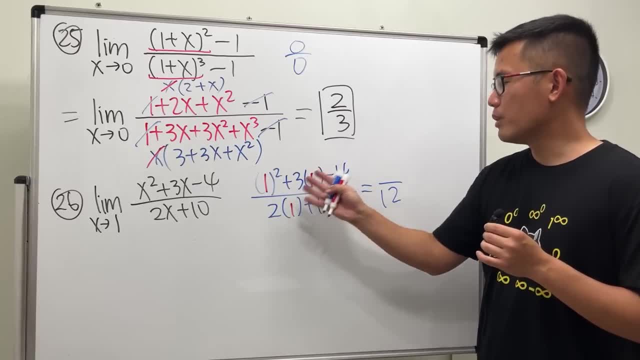 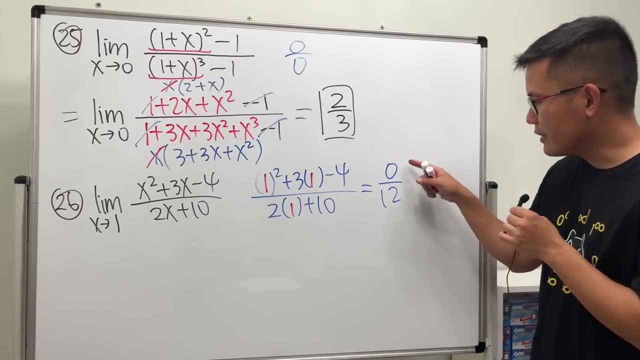 On the top. what do we get? 1 plus 3 is 4,. 4 minus 4 is 0. So we have 0 over 12.. Can we draw a conclusion? Yes, When we have a number, when we have a 0 over a non-zero number. 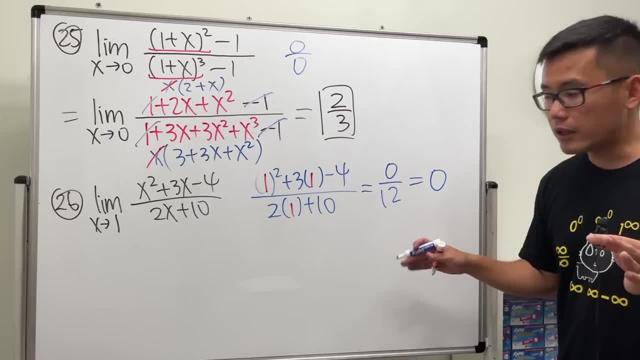 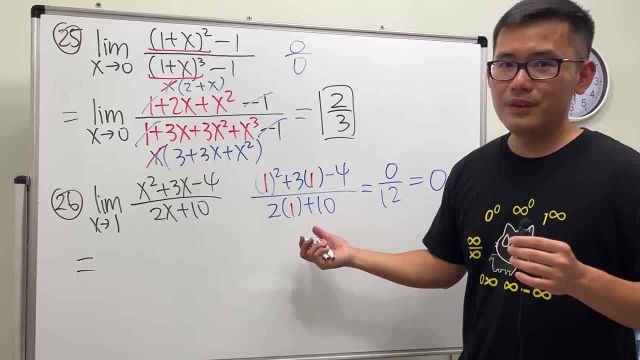 we can draw a conclusion, and the answer for that is 0. Done deal. So, in fact, the way that you can show work for this question is just plug it, because it does not give you a determinant form. However, the next answer is: that's it. 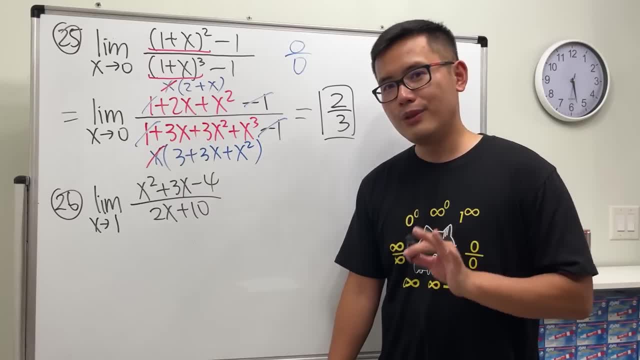 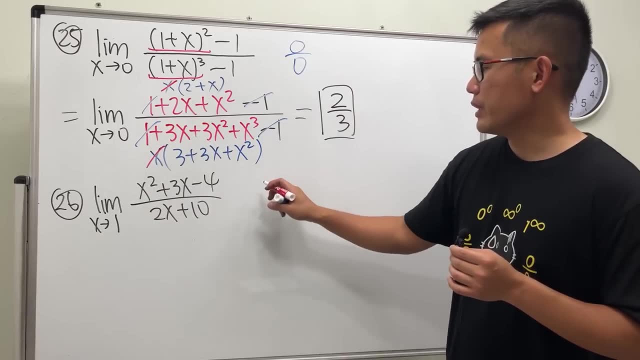 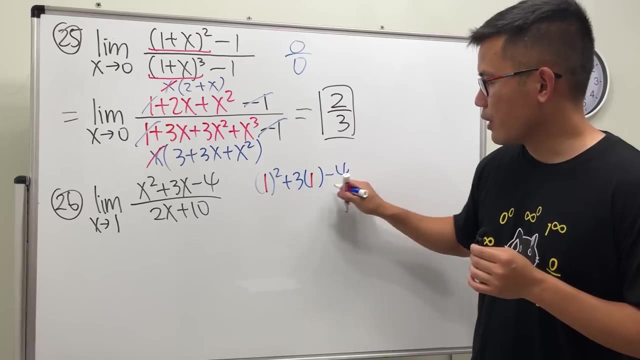 Go ahead and factor and try to cancel. No, No, No, Why Again have the good habit, Put the 1 into here. Let's see what we get. So we get 1 squared plus 3 times 1 and then minus 4, over 2 times 1 and then plus 10.. 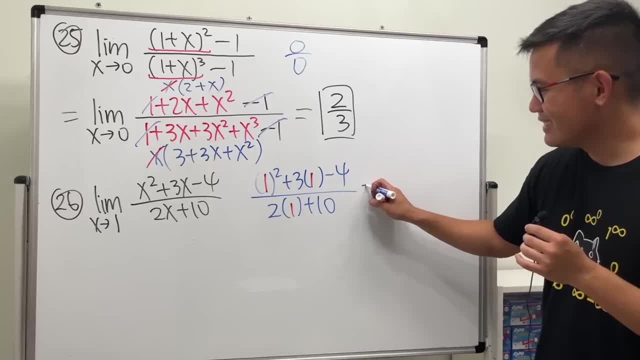 Do we get 0 on the bottom? No, we don't. huh, It's the 12 on the bottom. On the top, what do we get? 1 plus 3 is 4.. 4 minus 4 is 0.. 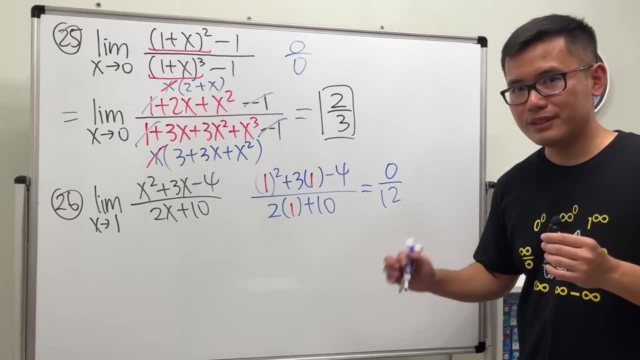 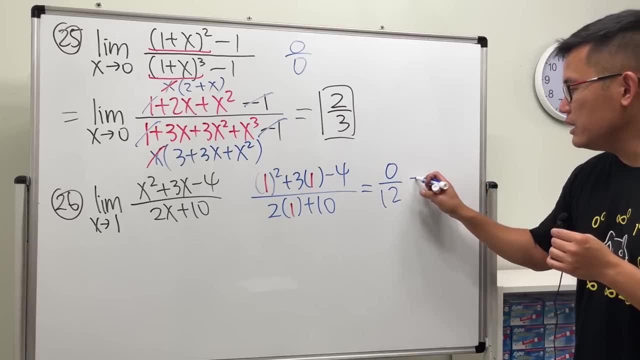 So we have 0 over 12.. Can we draw a conclusion? Yes, When we have a number, When we have a 0 over a non-zero number, we can draw a conclusion And the answer for that is 0.. Done deal. 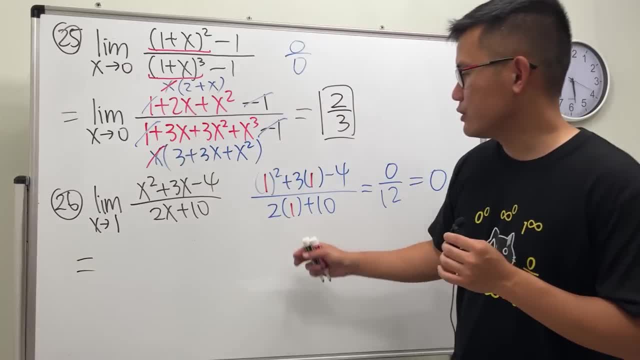 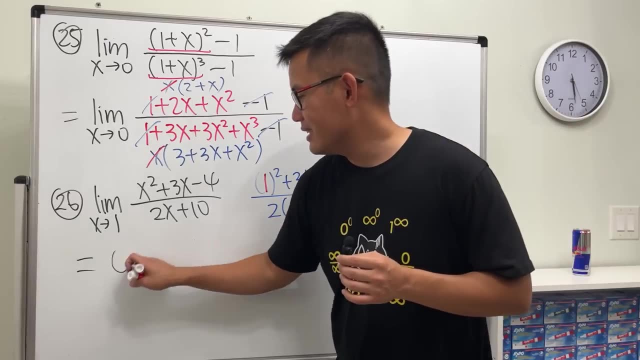 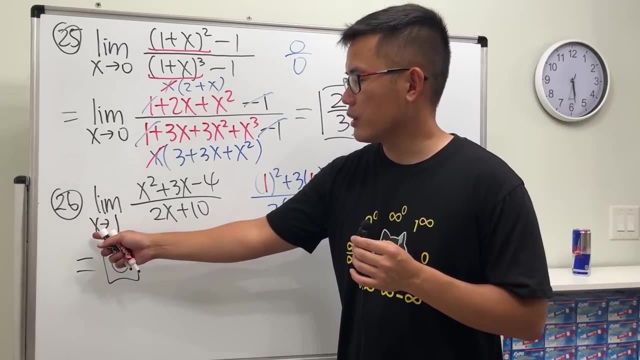 So, in fact, the way that you can show work for this question is just plug it, Because it does not give you a determinant form. However, the next answer is: that's it. Zero Done. Yeah, This question might be slightly more difficult if we are talking about x is approaching negative 5.. 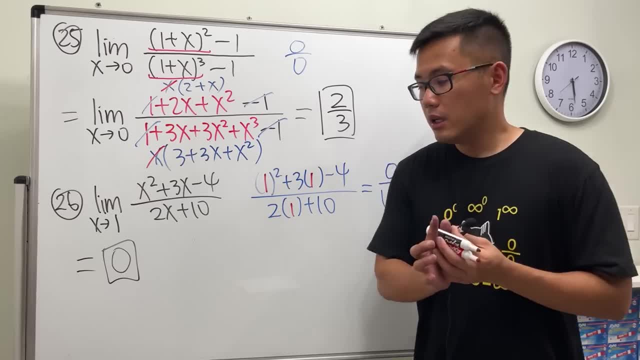 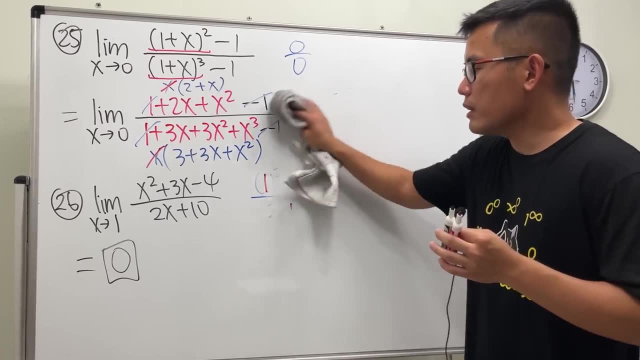 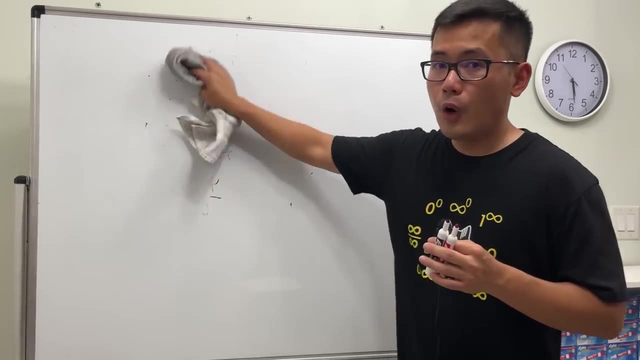 Because that will make the bottom 0. In that case you have to Investigate the left and also the right limit. But that wouldn't be a 0 for 0 either. So yeah, So for number 26,. it's just like a reminder that hey, don't forget to have the good habit that always plug in the value. 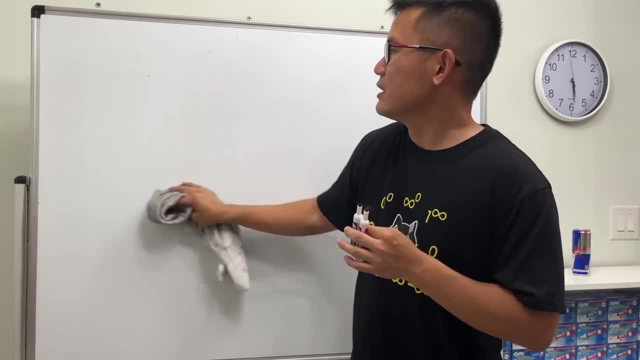 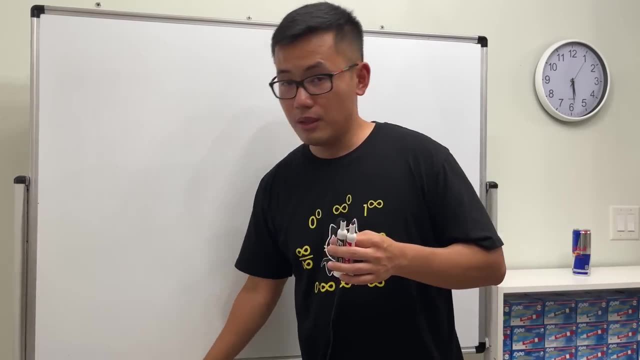 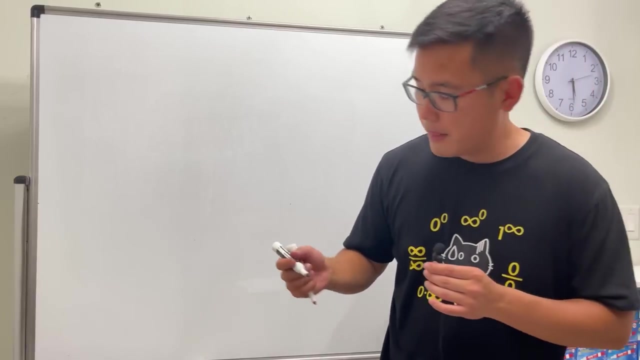 Because sometimes, when you do a lot of algebraic simplifications, it's like: huh, what do I have to do with that? Sometimes, simply plug in and then work that out. Maybe you are done already, So let's go to number 27.. 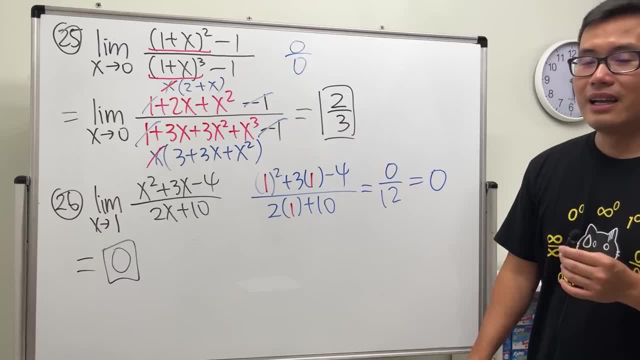 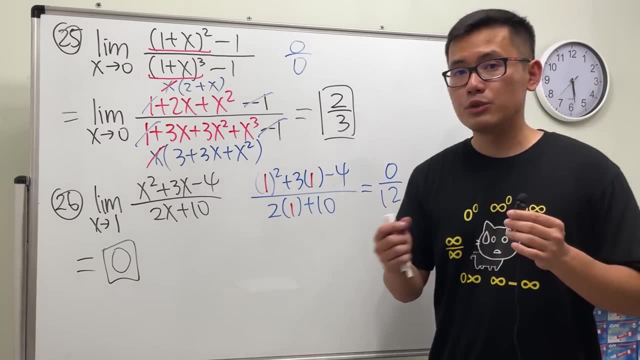 0. Done. Yeah, This question might be slightly more difficult if we are talking about x is approaching negative 5, because that would make the bottom 0. In that case you have to investigate the left and also the right. But that wouldn't be a 0 for 0 either. 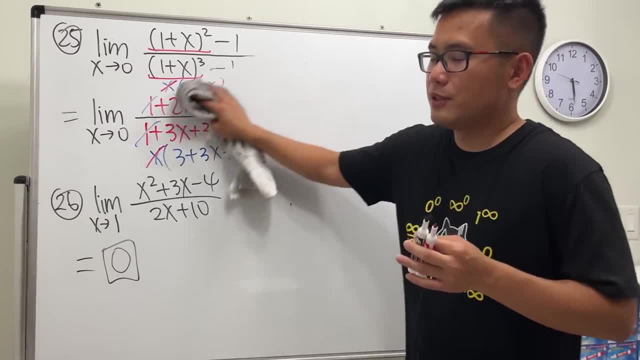 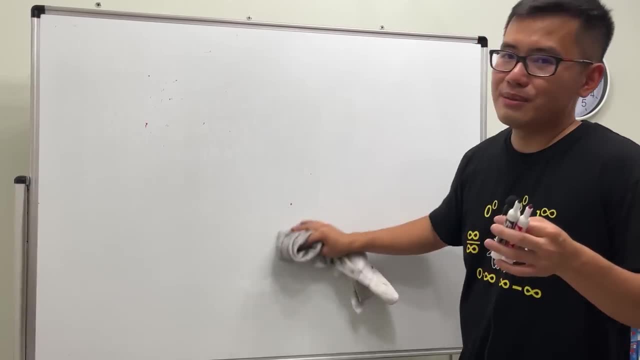 So for number 26,. it's just like a reminder that hey, don't forget to have the good habit that always plug in the value, Because sometimes when you do a lot of algebraic simplifications it's like: huh, what do I have to do with that? 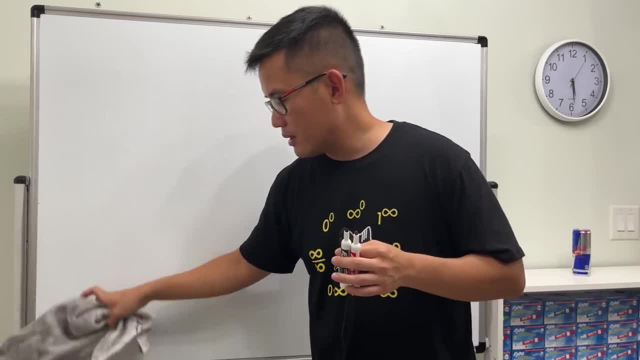 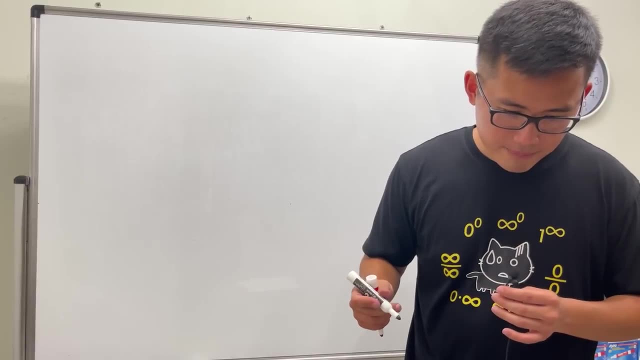 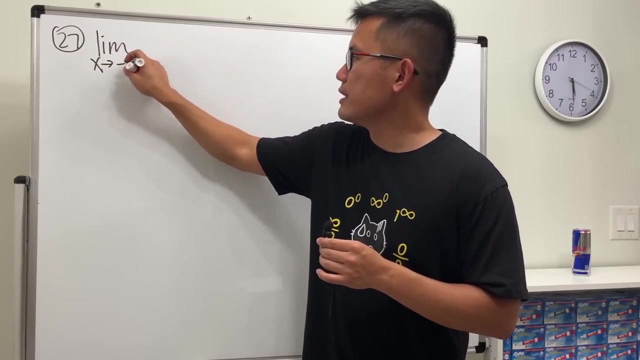 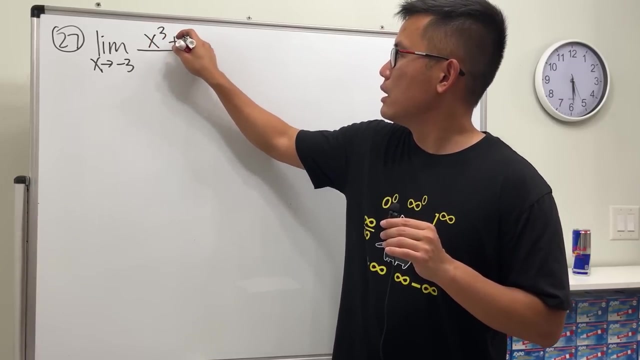 Sometimes simply plug in and then work that out. Maybe you are done already. 27,. here we have the limit as x approaching negative 3. And then we have x to the third power plus 27 over x plus 3.. So let's see. 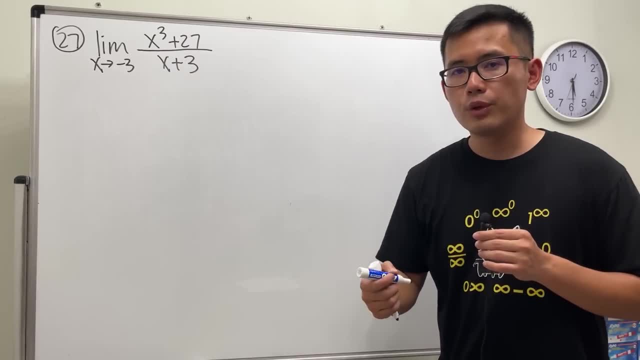 If we plug in negative 3, raise that to a third power, we get negative 27,. we get 0.. Plus 27,, so 0.. On the bottom we also get 0,, so 0 for 0.. 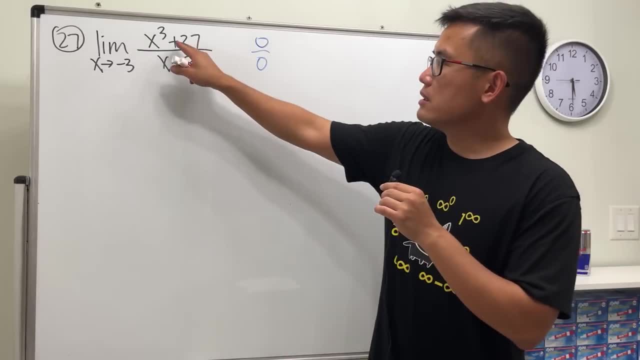 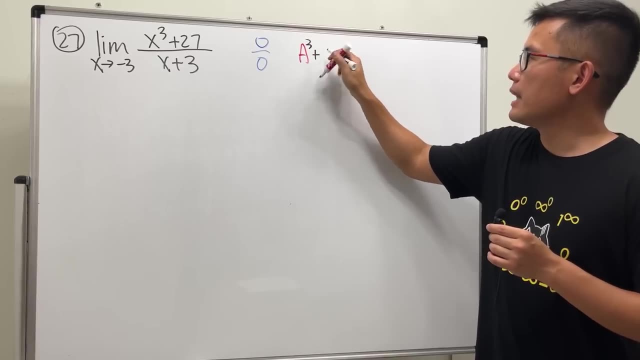 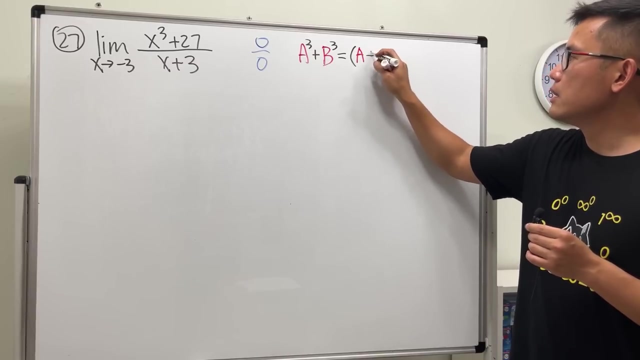 So how do we do it? This is a sum of two cubes, So I will remind you guys how to factor that When we have a to the third power plus b to the third power, the way to factor this is a plus b times a squared minus ab. 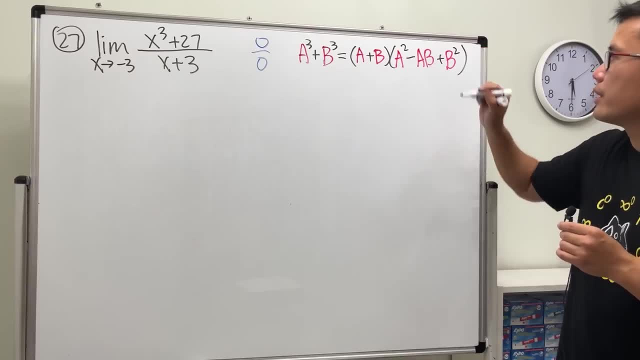 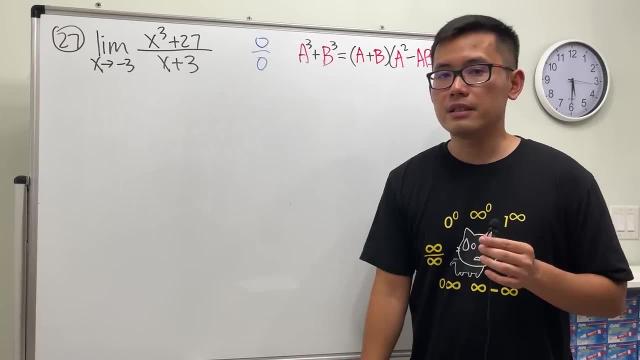 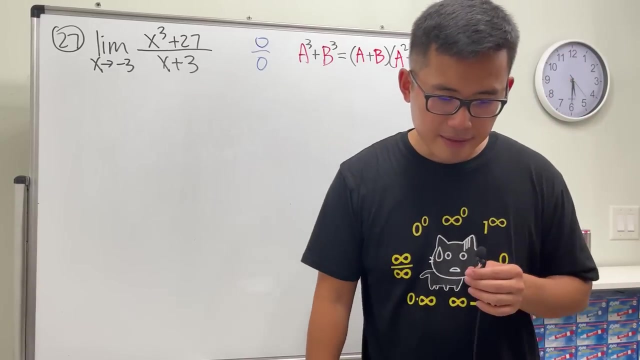 and then plus b squared, Okay, Okay, So in this particular case you can also do polynomial long diffusion or synthetic diffusion. I think both of them will work out okay. But let me show you guys how to factor this, because I have the synthetic diffusion equation for number 28.. 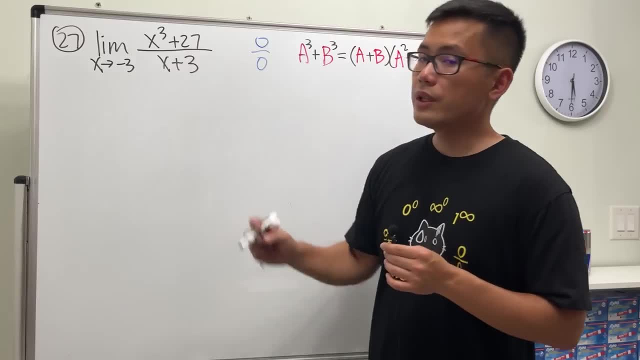 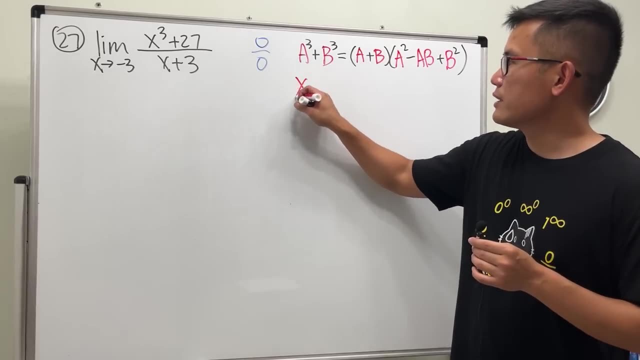 So for this one, let's factor it. So notice: 27 is the same as 3 to the third power, So I'm just perhaps going to write it right here. So we have x to the third power plus 3 to the third power. 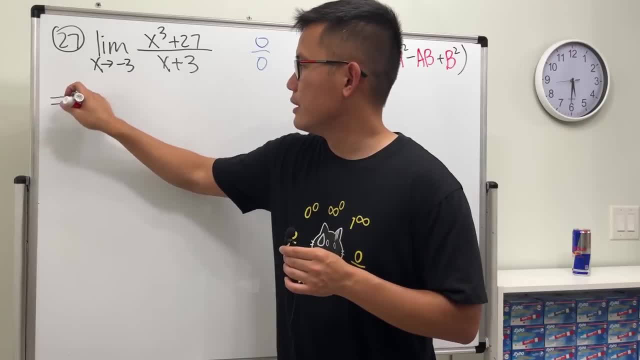 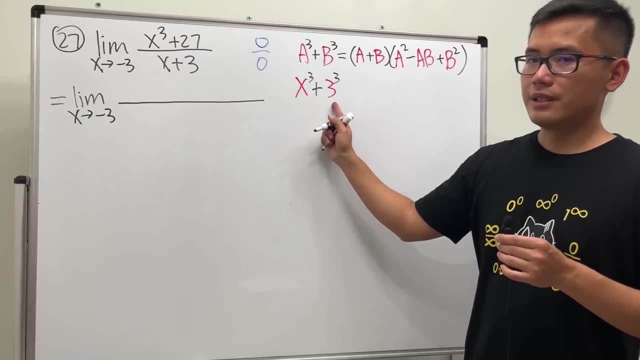 And then we can just draw in. But let me put down the result right here. So this is the limit as x approaching negative 3.. So this right here, just look, We will have x plus 3.. That's the first factor. 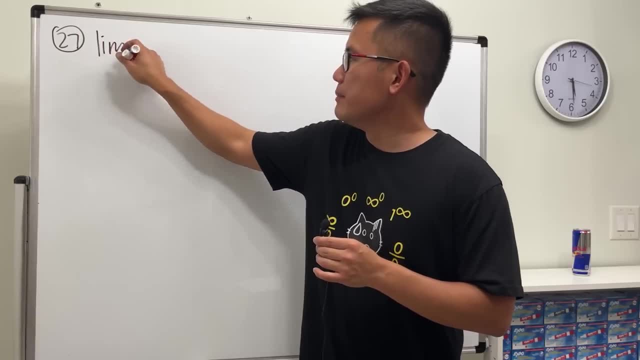 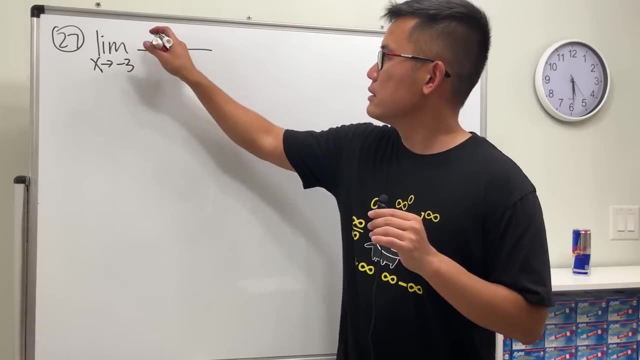 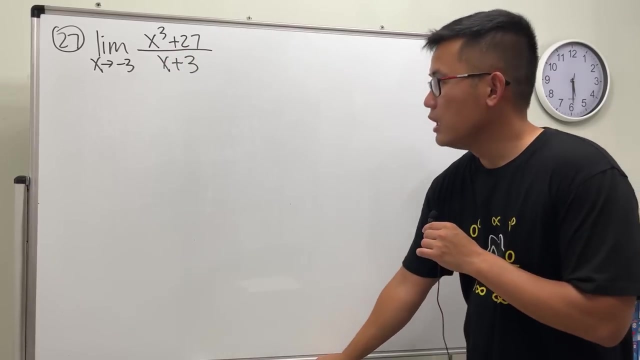 27.. Here we have the limit as x approaching negative 3. And then we have x to the third power plus 27.. Over x plus 3.. So let's see, If we plug in negative 3, raise that to the third power, we get negative 27.. 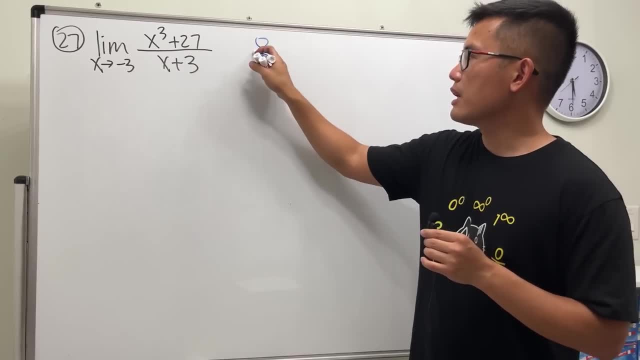 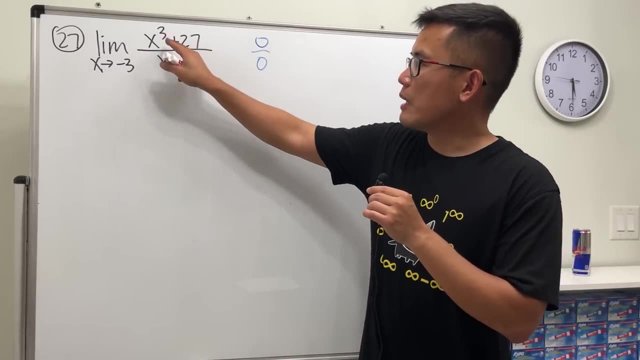 We get 0., Right Plus 27,, so 0.. On the bottom we have to plug in negative 3. also get zero, so zero for zero. how do we do it? this is a sum of two cubes, so i will remind you. 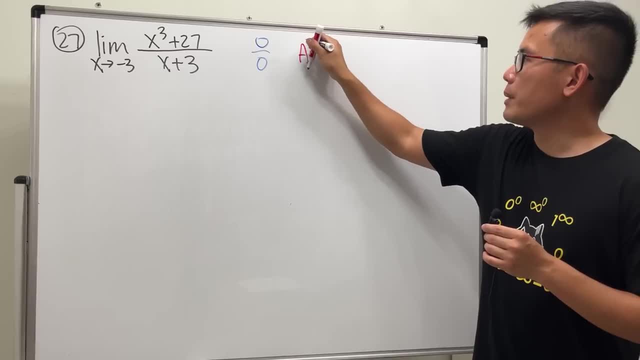 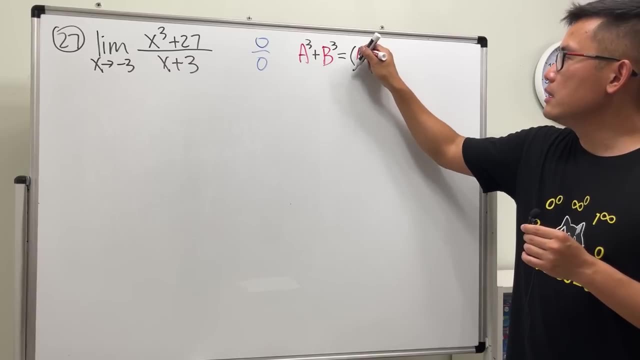 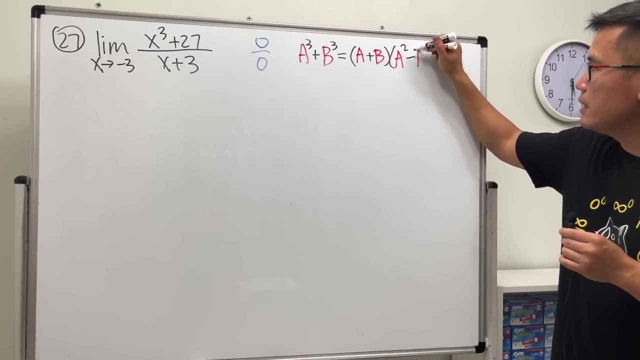 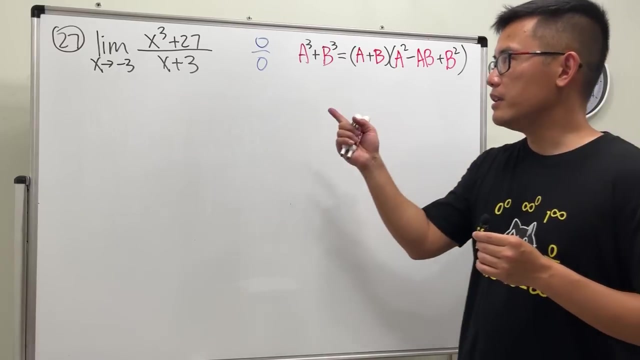 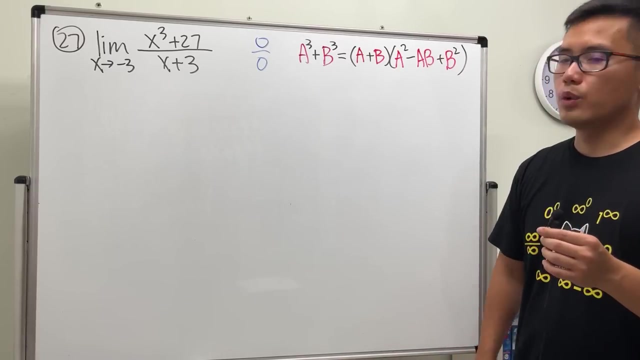 guys how to factor that when we have a to the third power plus b to the third power. the way to factor this is a plus b times a square, minus a b and then plus b square, okay. and in this particular case you can also do polynomial long diffusion or synthetic diffusion. i think both of them will work out okay, but let 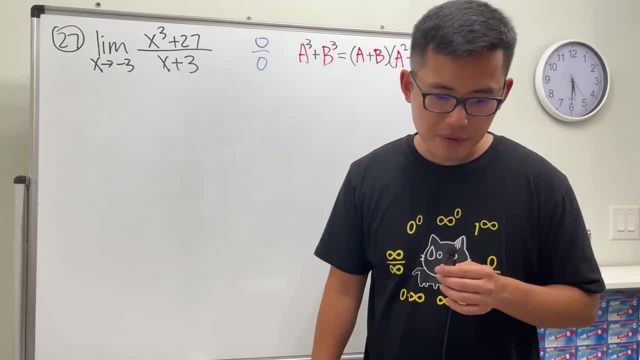 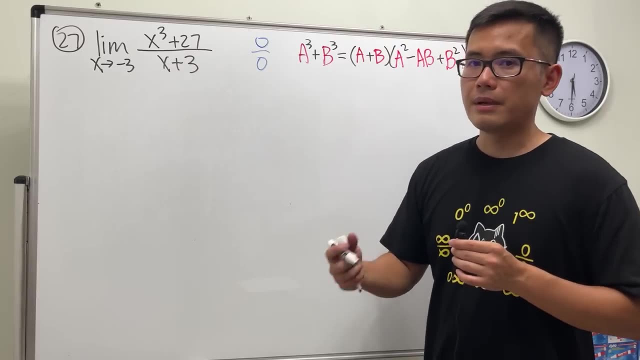 me show you guys how to factor this, because i have the synthetic diffusion question for number 28.. so for this one let's factor it. so notice: 27 is the same as 3 to the third power. so i'm just perhaps going to write it right here. 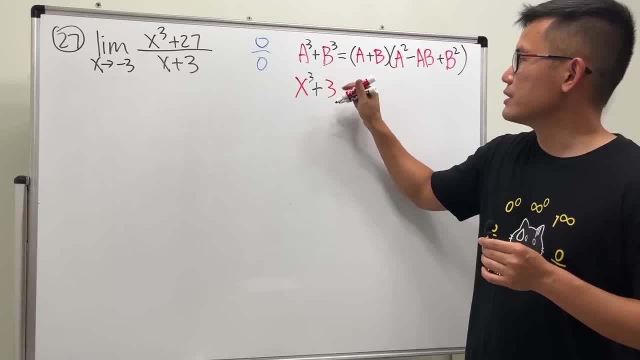 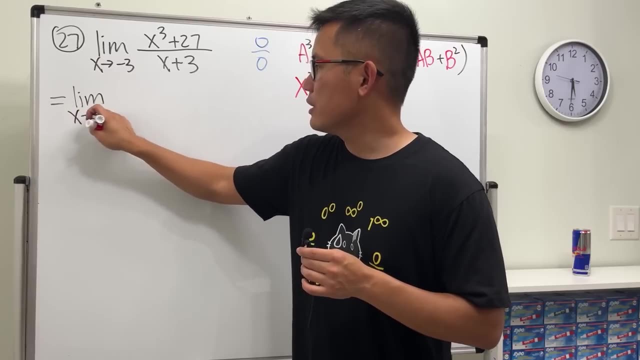 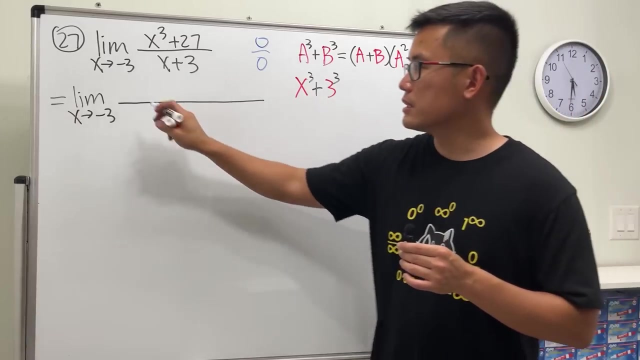 so we have x to the third power plus 3 to the third power, and then we can just draw in. but let me put on the result right here. so this is the limit as x approaching negative 3. so this right here, just look, we will have x plus 3. that's the first factor. so x plus 3. 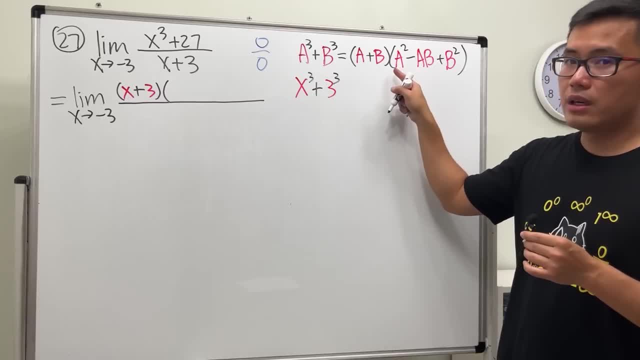 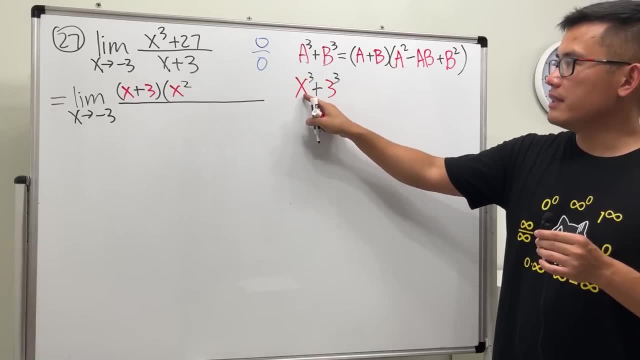 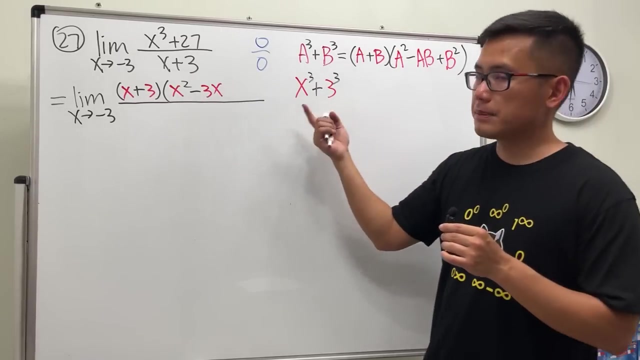 to continue, we will have x square, so let me just write it down: x square minus a, b, in this case minus x times 3, so that's minus 3x. lastly, plus b squared, and that's plus 3 squared, so that will give us 9.. 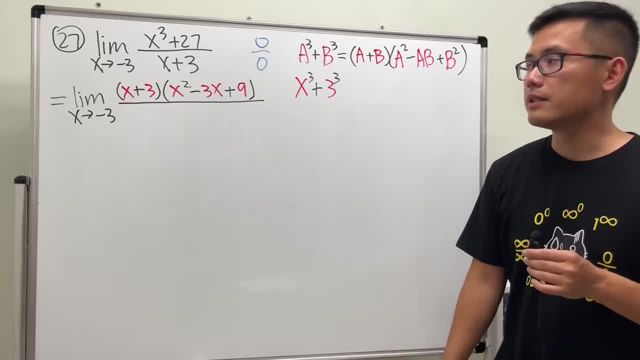 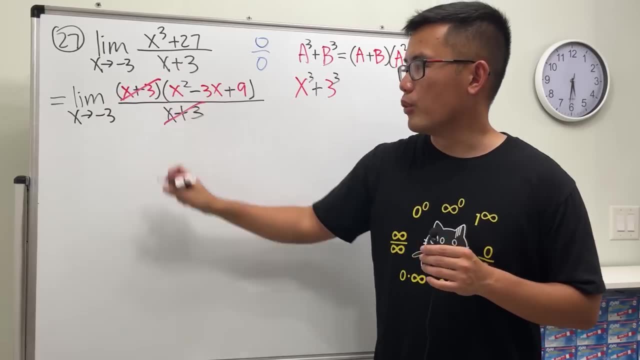 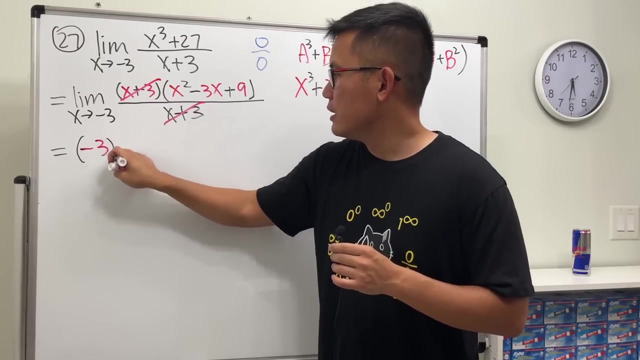 so that's the factoring for x to the third power plus 27.. on the bottom we still have the x plus 3. guess what? zero over zero, no more. then put the negative 3 into all the x's. we are going to get negative 3 square minus 3 times negative 3, and then plus 9.. 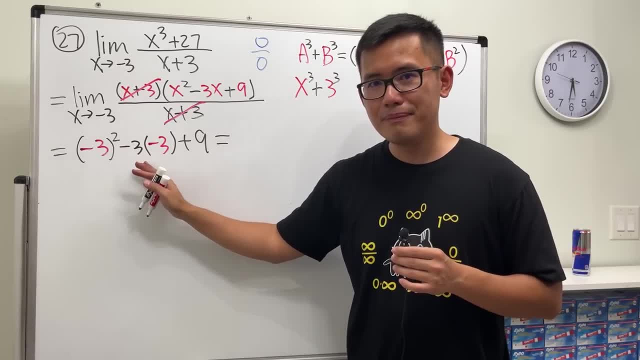 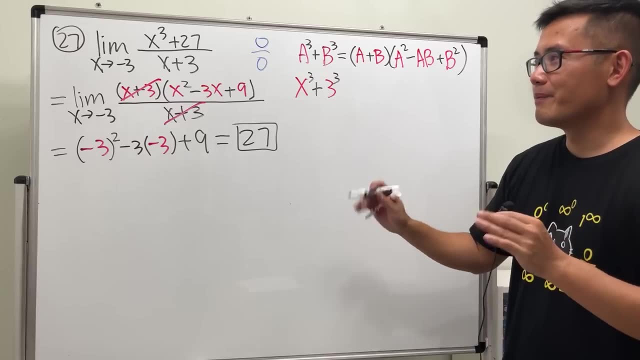 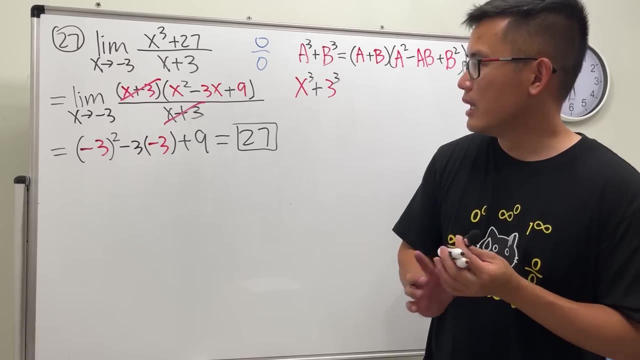 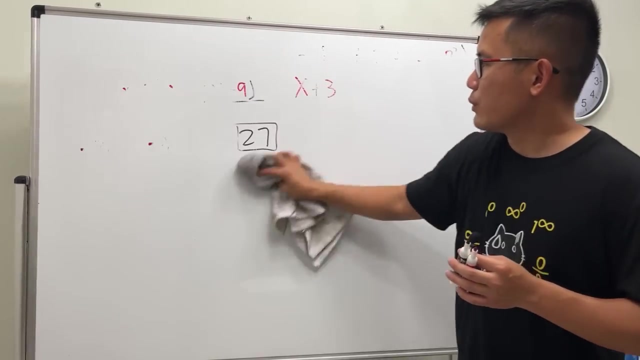 this is 9, another 9, another 9, 27.. yeah, code very is a pure constant that you get 27.. so for number 28, i'm going to show you guys the synthetic division and also the long division together. so i'm just going to erase this so that we have the whole board to show you guys both. 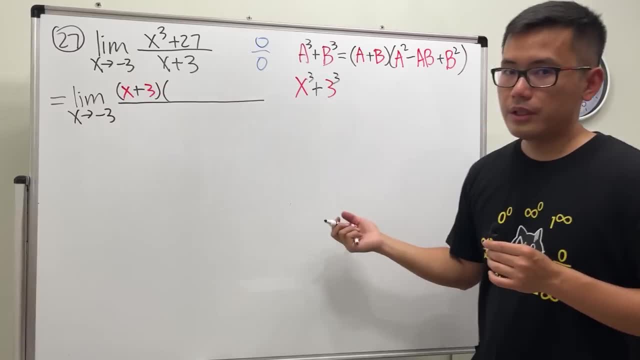 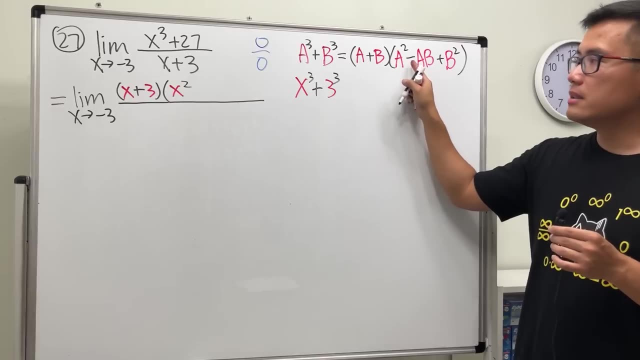 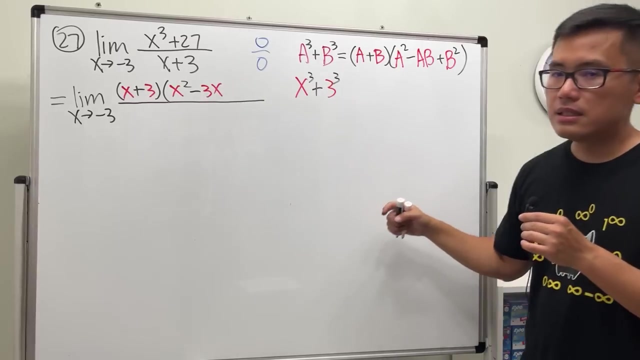 So x plus 3.. To continue, we will have x squared. So let me just write it down: x squared minus ab, In this case minus x times 3.. So that's minus 3x. Lastly, plus b squared. 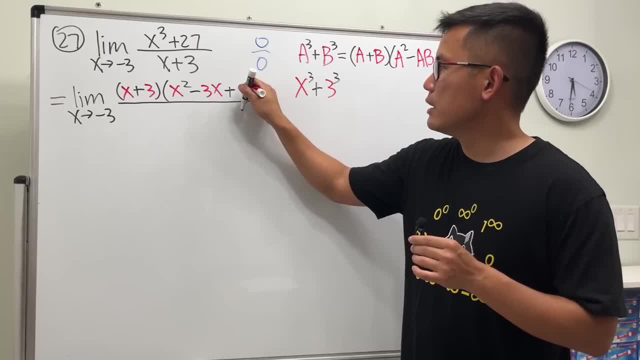 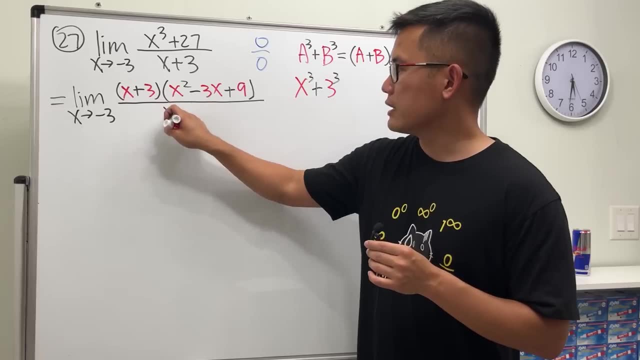 And that's plus 3 squared, So that will give us 9.. So that's the factoring for x to the third power plus 27.. On the bottom we still have the x plus 3.. Guess what? 0 over 0, no more. 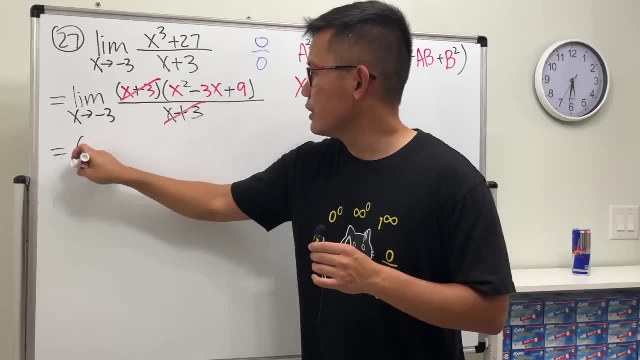 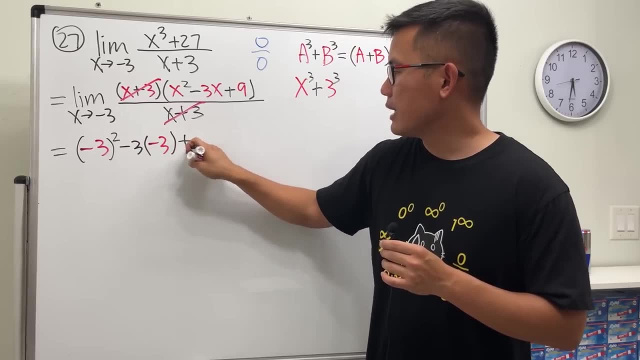 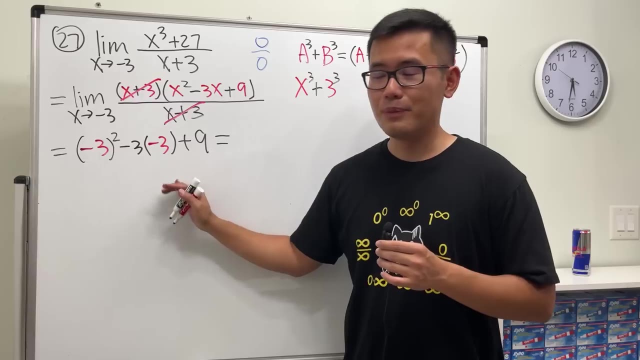 Then put the negative 3 into all the x's, We are going to get negative 3 squared minus 3 times negative 3. And then plus 9.. This is 9.. Another 9.. Another 9. 27. 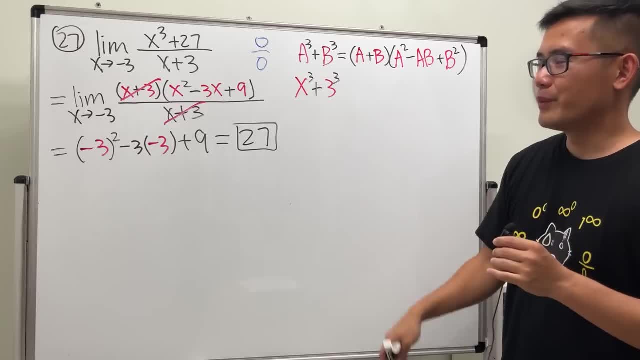 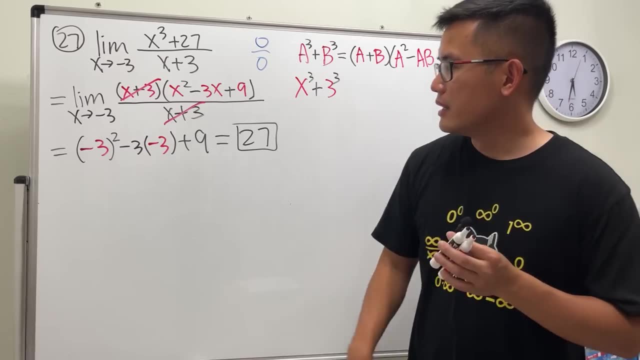 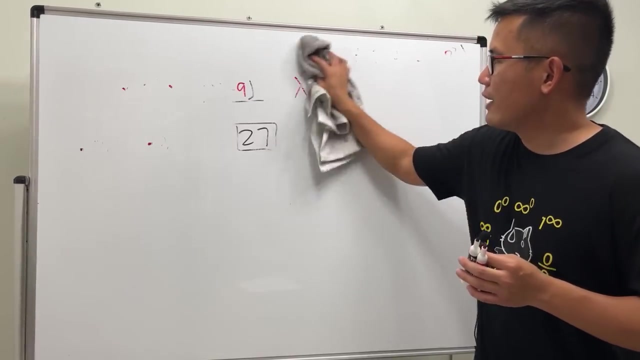 Yeah, very, it's a pure coincidence that you get 27.. All right, For number 28,. I'm going to show you guys the synthetic division and also the long division together. So I'm just going to erase this. So that way I have the whole board to show you guys. 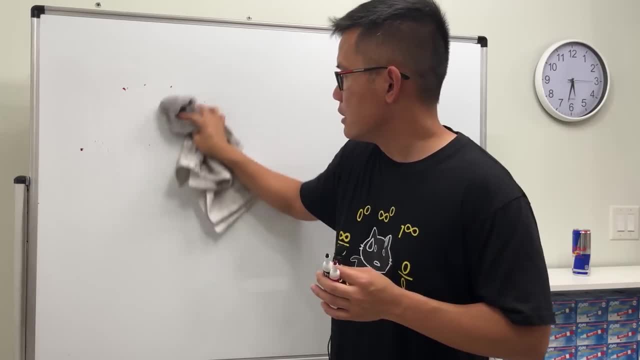 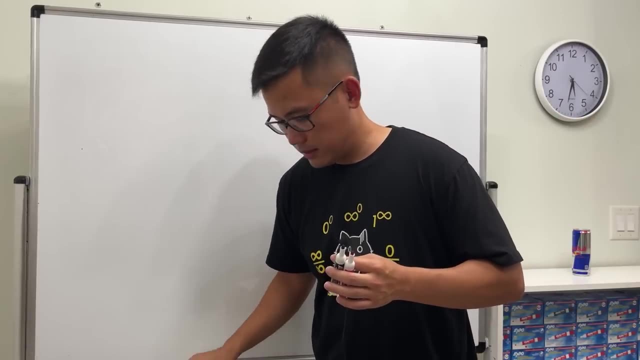 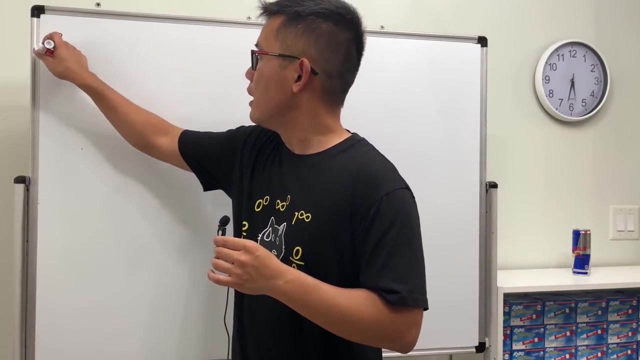 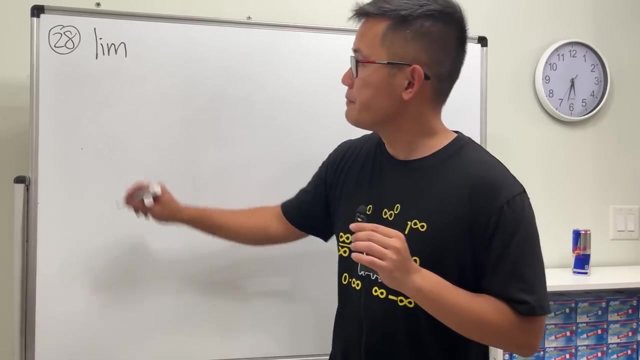 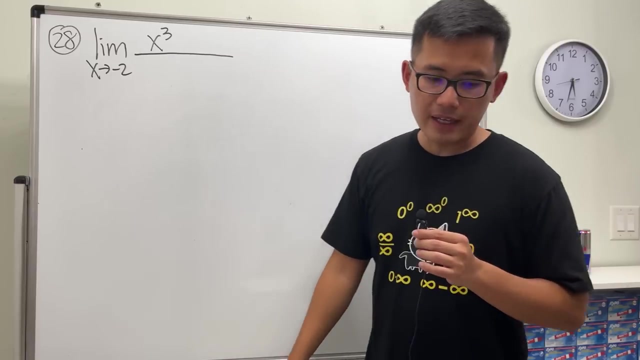 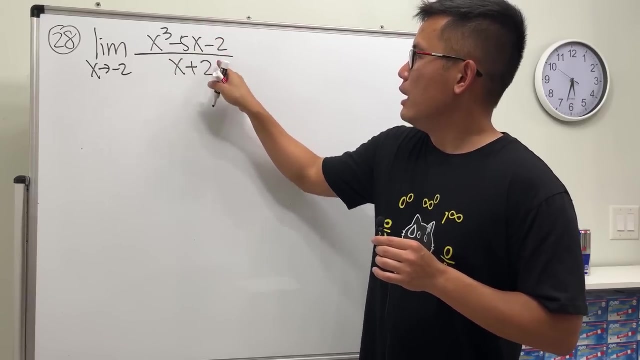 Both All right. For number 28, we have the limit as x approaching negative 2.. And we have x to the third power Minus 5x minus 2.. Over x plus 2.. As you can see on the top, we have a trinomial. 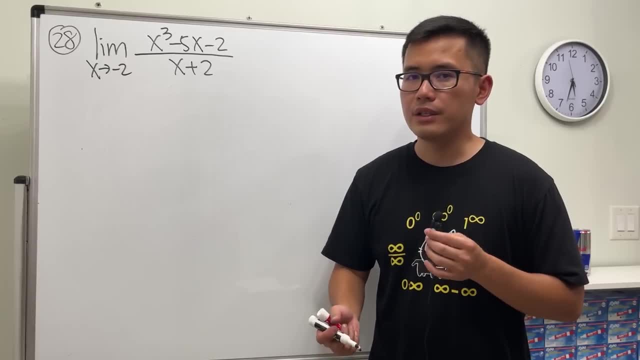 However, it's a cubic, It's not quadratic, So it's not that easy to factor it the usual way. But again, let's have a good habit: Plug in negative 2 into here. Negative 2 to the third power, we get negative 8.. 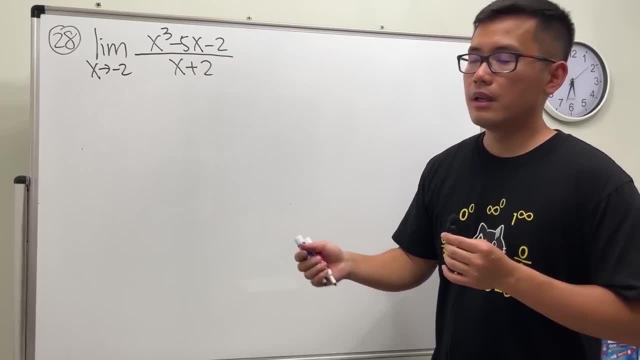 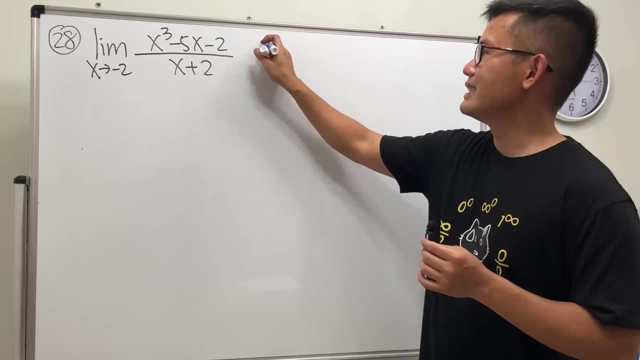 Plug into here. Negative 5 times negative 2 is 10.. Negative 8 plus 10 is negative. Negative 8 plus 10 is negative. Negative 8 plus 10 is 2.. Minus 2, we get 0.. 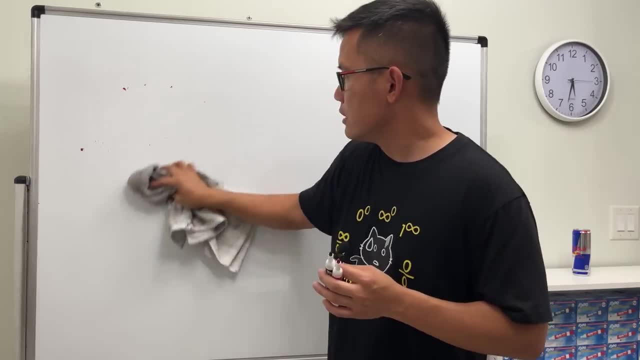 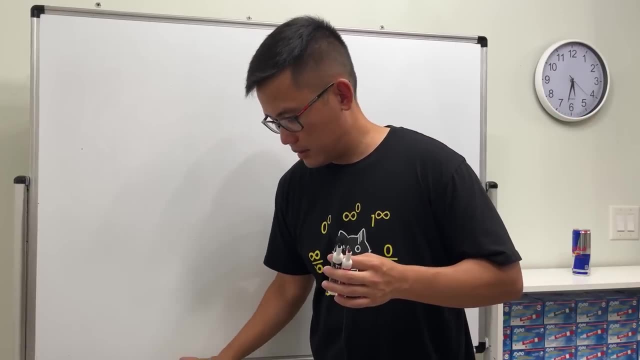 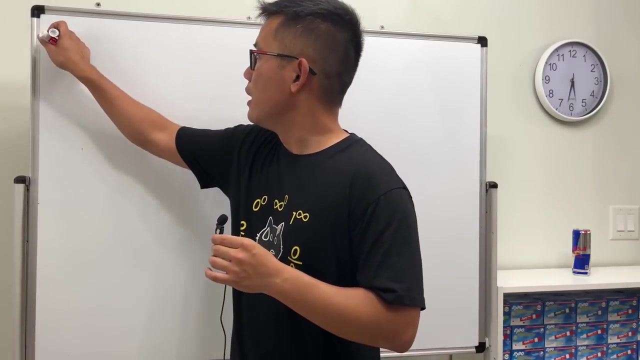 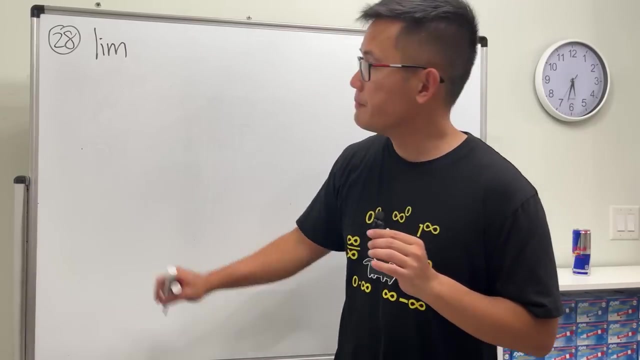 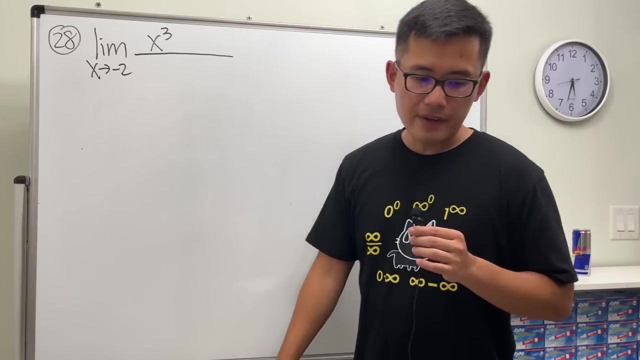 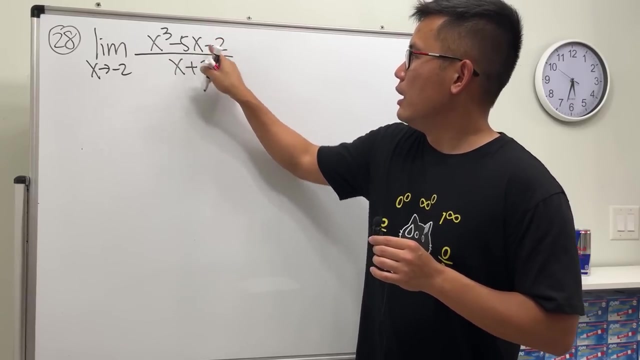 so all right. for number 28, we have the limit as x approaching negative 2 and we have x to the third power minus 5x, minus 2 over x plus 2. as you can see on the top, we have a trinomial. however, it's a cubic, it's not quadratic. 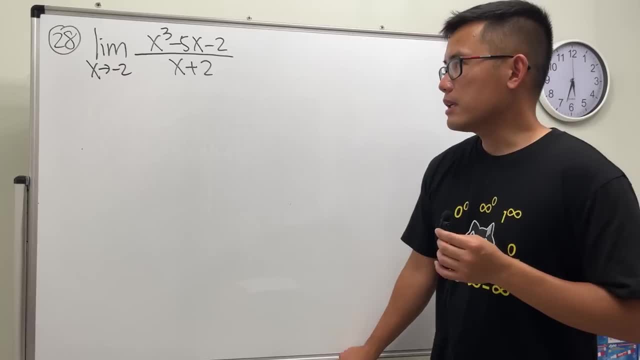 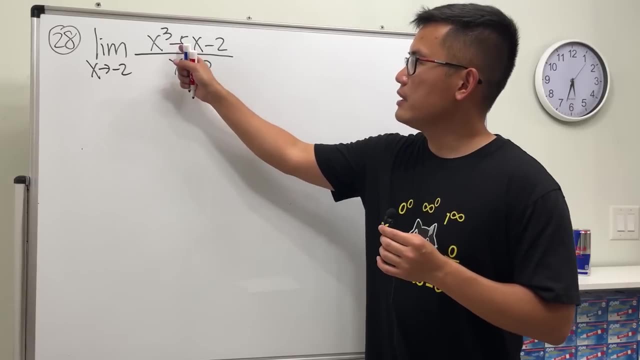 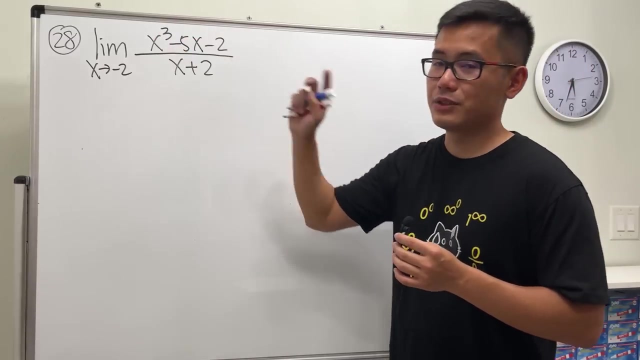 so it's not that easy to factor it the usual way. but again, let's have a good habit. plug in negative 2 into here negative 2 to third power, we get negative 8. plug into here negative 5 times negative. 2 is 10 negative. 8 plus 10 is negative. negative. 8 plus 10 is 2 minus 2, we get 0. likewise, put a. 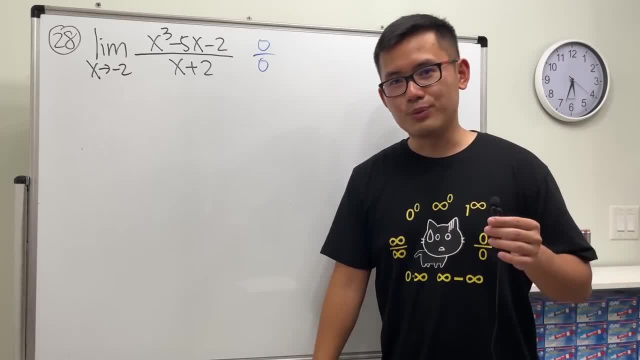 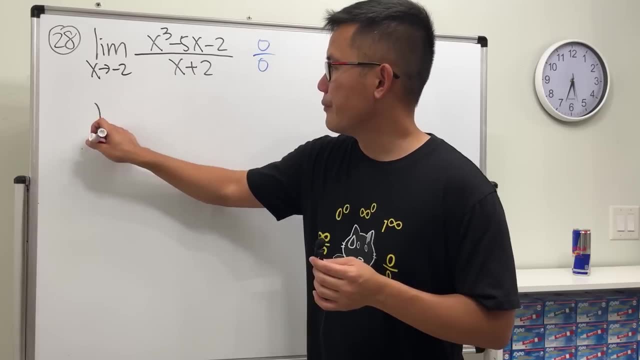 negative 2. here we also get 0, so 0 over 0. let's do more work. so the first thing is that we can just do polynomial long division you, and to do so i'm just going to put it inside here: x to the third power, and then we see we do not have 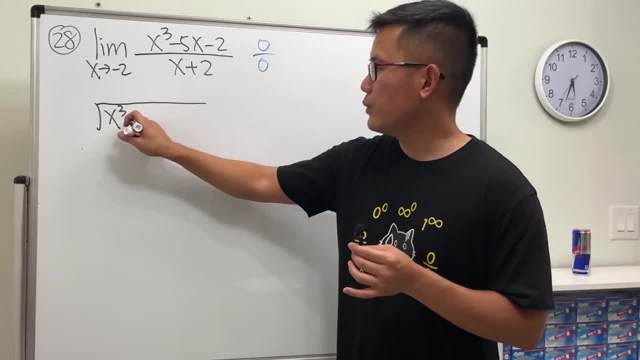 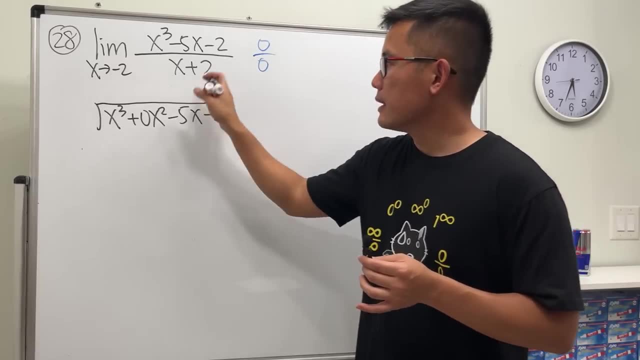 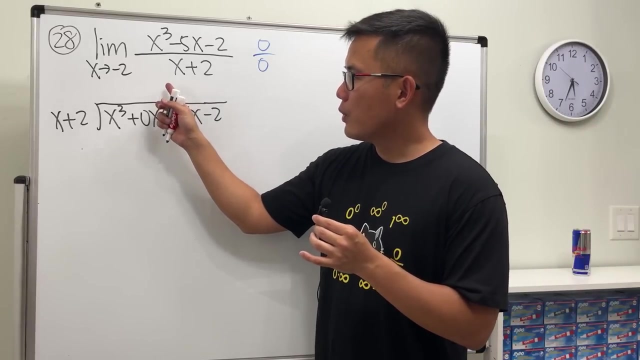 the quadratic term right. so i'm just going to say we have plus 0, x squared, and then minus 5x and then minus 2, and then here we have the x plus 2 on the outside. all right, so now we have to ask ourselves what times x will give us x to the third power. the answer is x squared, so put the result. 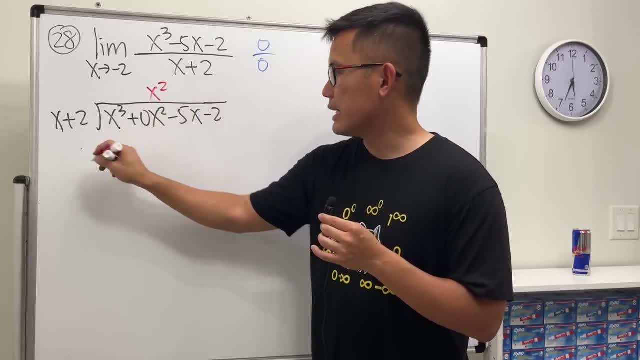 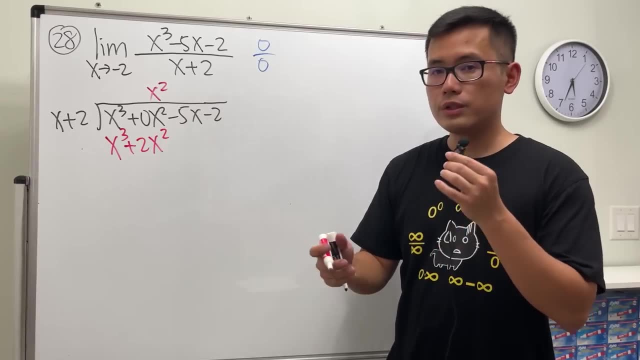 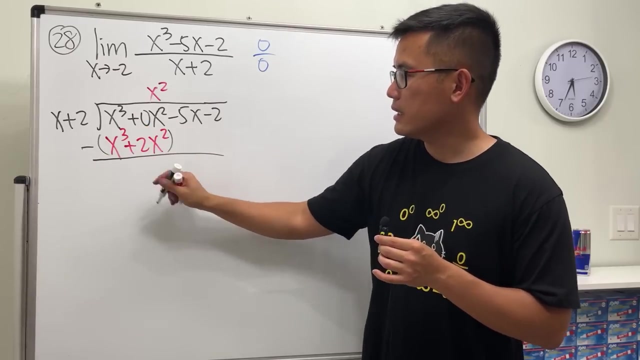 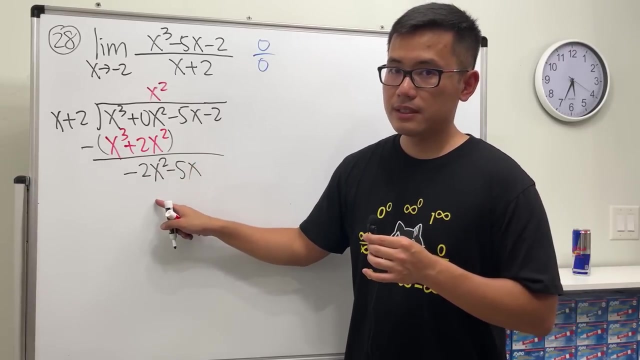 line up right here x square times. that gives us x plus third power. take this times that we get plus 2x square and when we do long division we subtract. so this: right here we have this: this minus 0, 0, minus that we get negative 2x squared. bring down the negative 5x. what do we do next? here we have x. 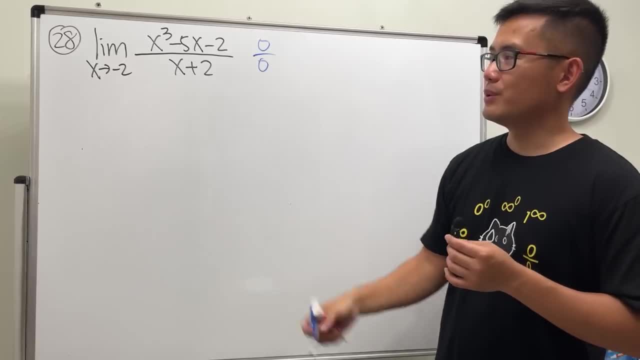 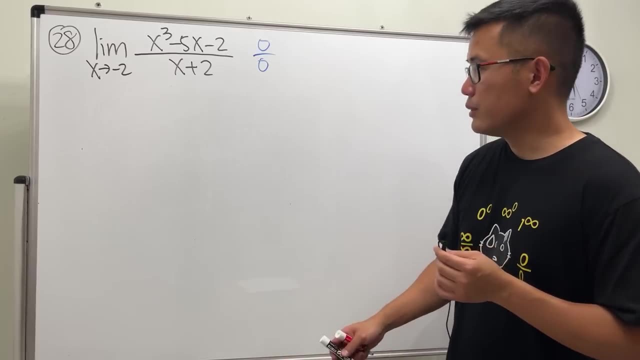 Likewise put the negative 2 here we also get 0.. So 0 for 0.. We have to do more work. So the first thing is that we can just do polynomial long division, And to do so- I'm just going to put it inside here: x to the third power. 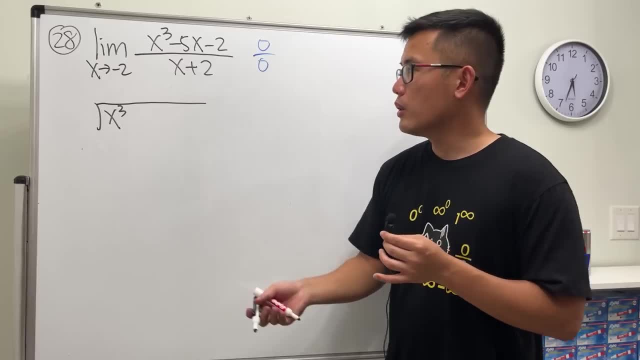 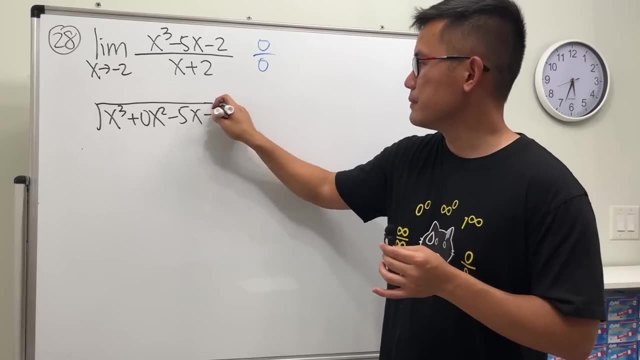 And then we see we do not have the quadratic term right. So I'm just going to say we have plus 0x squared, And then minus 5x, And then minus 5x And then minus 2.. And then here we have the x plus 2 on the outside. 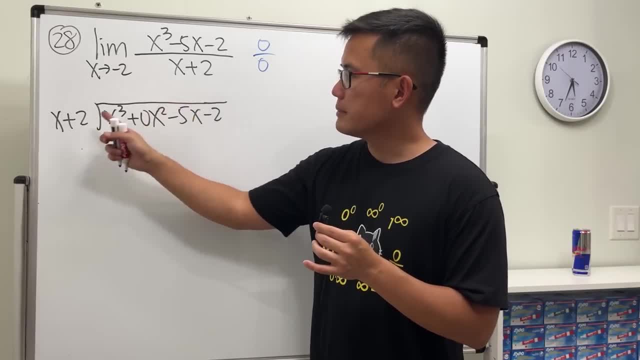 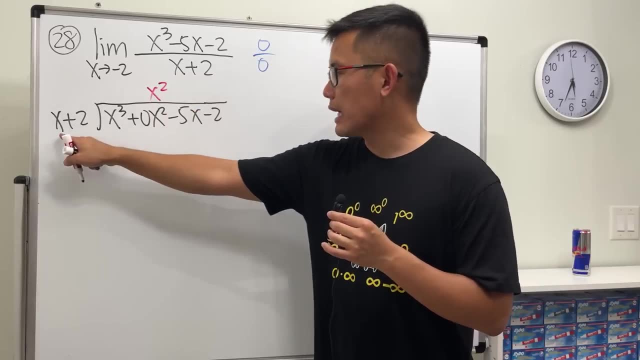 All right. so now we have to ask ourselves what times x will give us x to the third power. The answer is x squared, So I'll put the result lined up right here: x squared times. that gives us x to the third power. 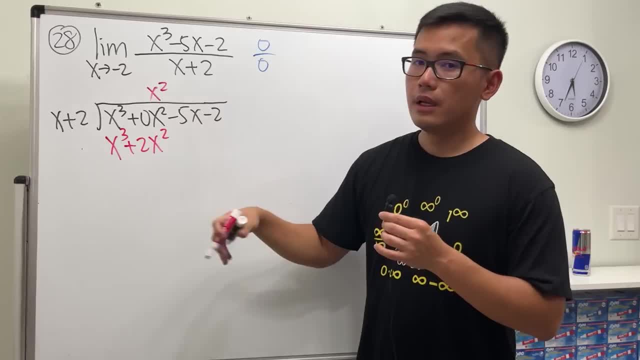 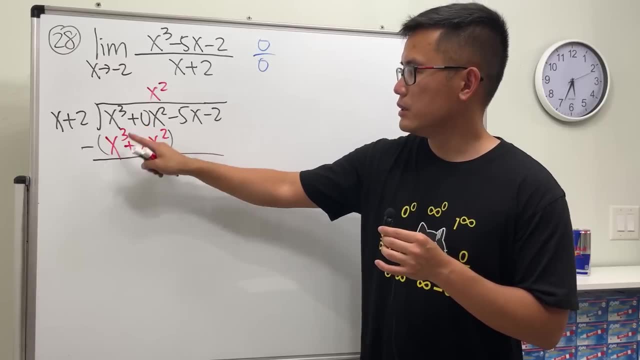 Take this times that we get plus 2x squared And when we do long division we subtract. So this right, here we have this: This minus 0.. This minus 0.. 0 minus that we get negative 2x squared. 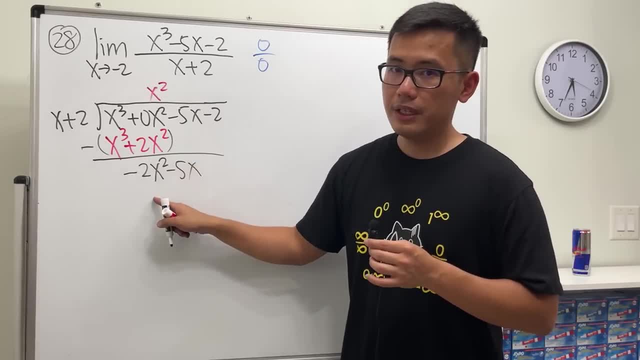 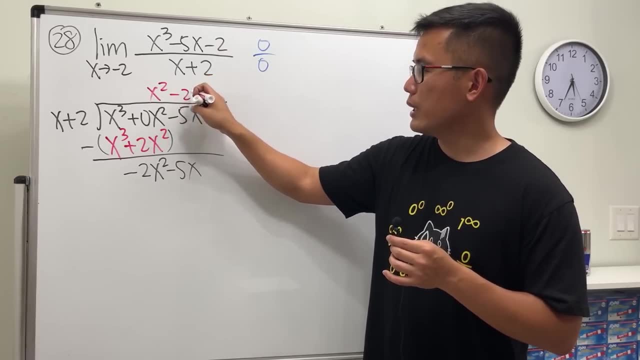 Bring down the negative 5x. What do we do next? Here we have x. We need to get negative 2x squared. So we need negative 2x. Take that, multiply by this: we get negative 2x squared. 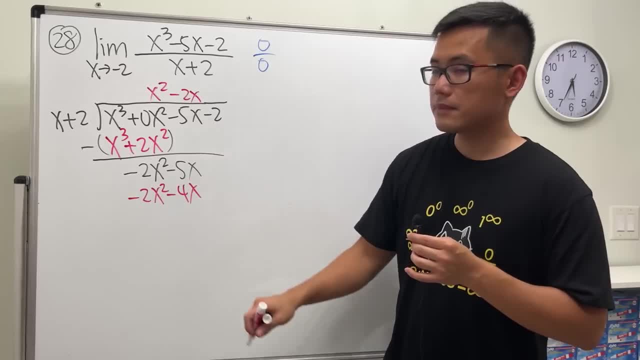 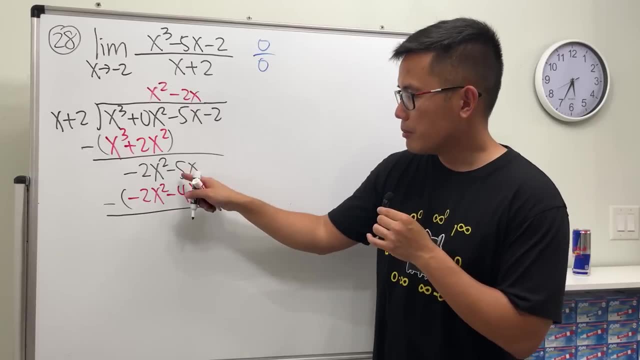 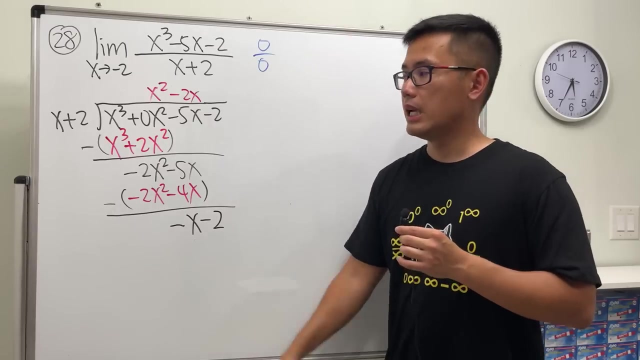 Take that, multiply by that we get negative 4x. All right, subtract Negative: 5 minus minus become plus, So negative. 5 plus 4 is negative, and then we have the x, And then we have that minus 2.. 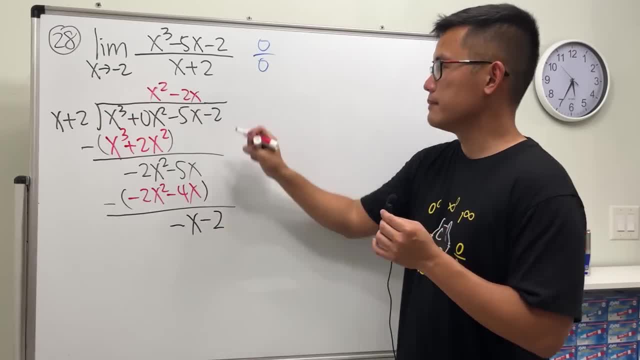 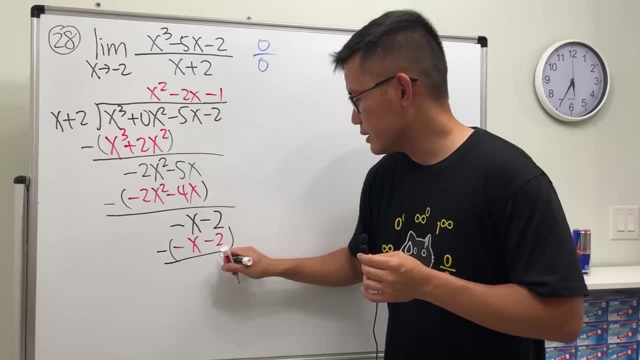 This is x plus 2.. We need that, so we need negative 1.. So put a negative 1, multiply we get negative x minus 2.. Subtract we get 0. Cool. So, with this being done, this right here tells us we just have to compute. 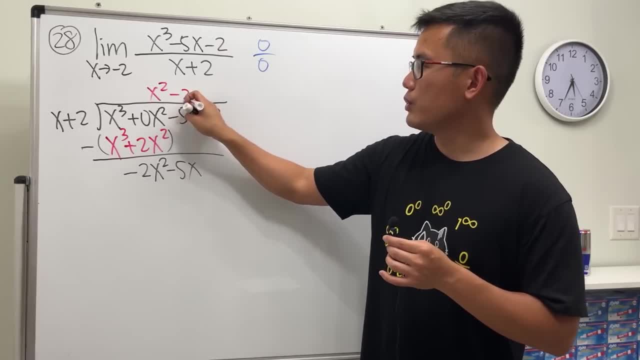 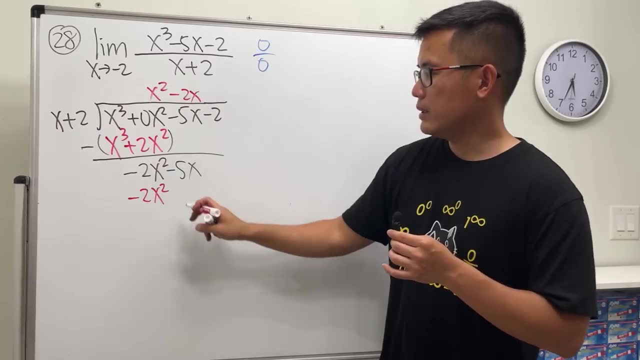 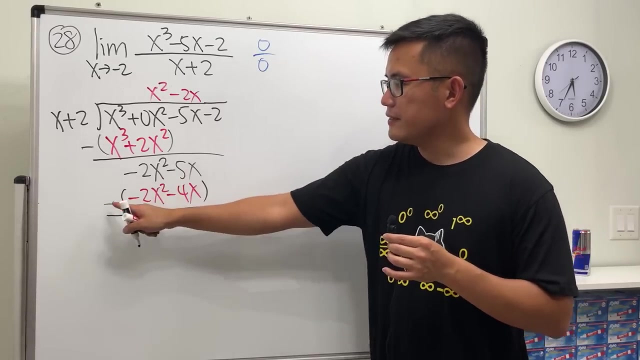 we need to get negative 2x squared. so we need negative 2- 2x. Take that, multiply by this: we get negative 2x squared. Take that, multiply by that, we get negative 4x. All right, subtract Negative 5, minus minus become plus. So negative 5 plus 4. 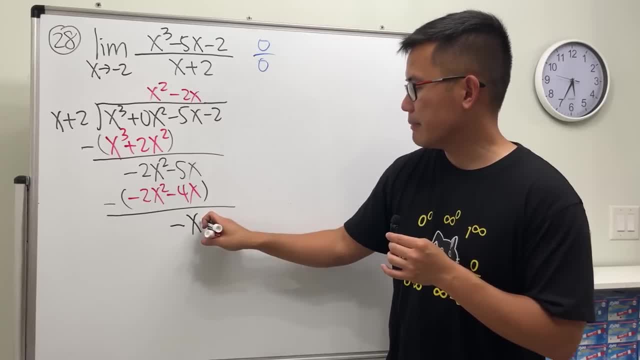 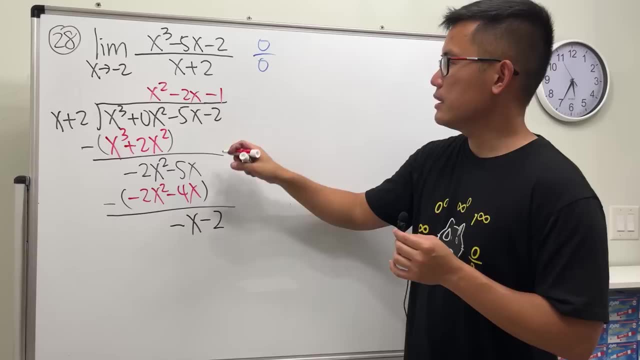 is negative, and then we have the x, and then we have that minus 2.. This is x plus 2. We need that, so we need negative 1. So put a negative 1, multiply, we get negative x minus 2.. Subtract. 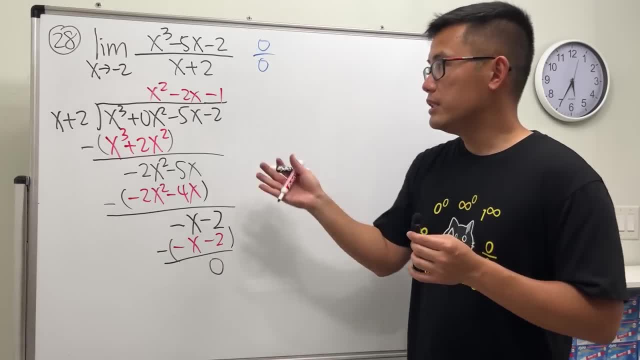 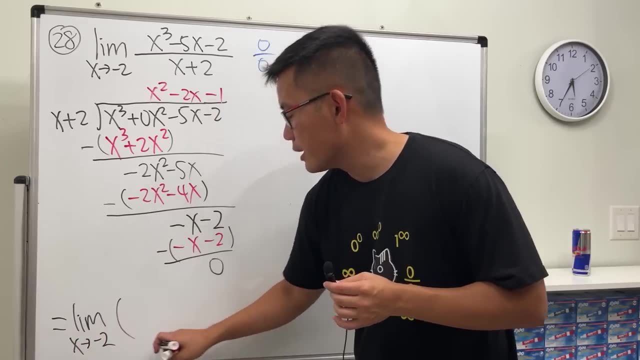 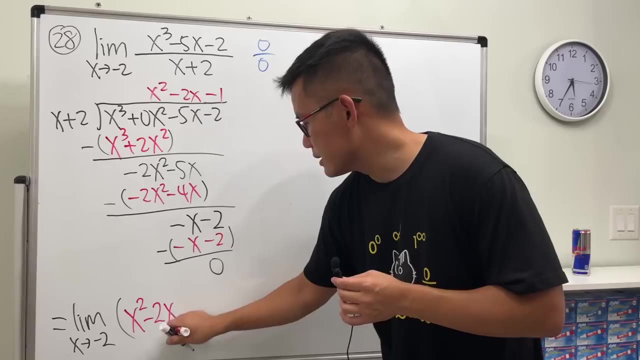 we get 0.. Cool. So, with this being done, this right here tells us we just have to compute the limit as x approaching negative 2.. The whole thing reduces to that, and that's x squared minus 2x minus 1.. So what we can do at the end. 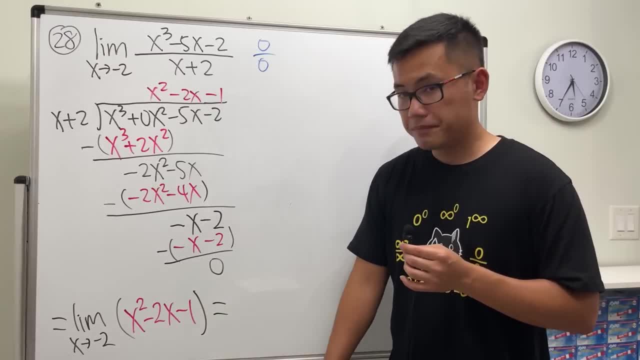 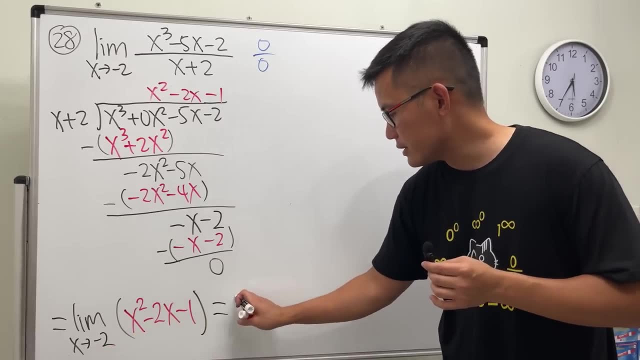 just go ahead and plug in negative 2.. So negative 2 in, here we get 4, and then plus another 4 is 8, and then minus 1 is 7.. So the answer for this is 7.. All right, so last one, just you plug in. 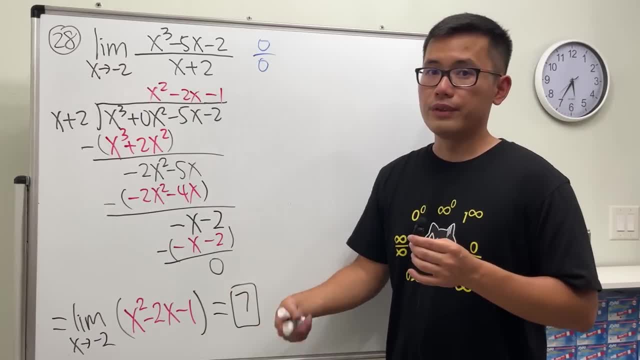 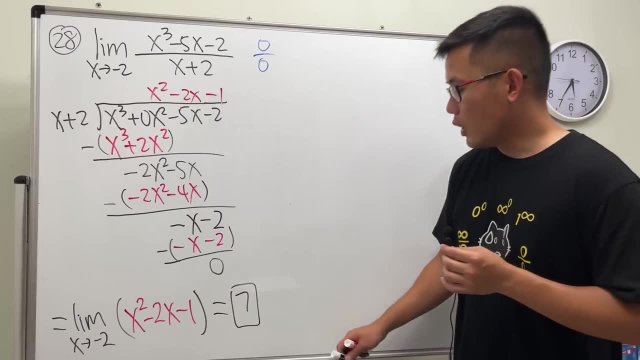 then you evaluate. So this is another way to cancel out the 0 for 0, right, Because the x minus 2 is gone. Yeah, Okay. so how do we do the so-called synthetic diffusion? then Here's the deal. 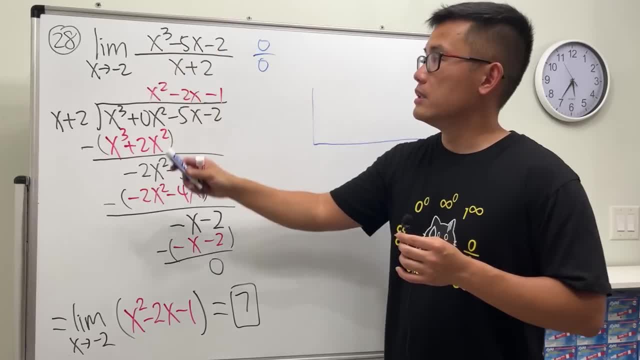 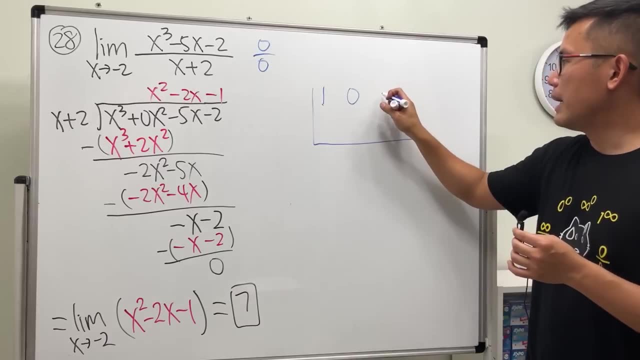 Look at the coefficients, So starting with 1,, and we do not have the x squared term, so just 0, and then minus 5, and then minus 2,. right The same, right here: 1, 0, negative 5,, negative 2.. 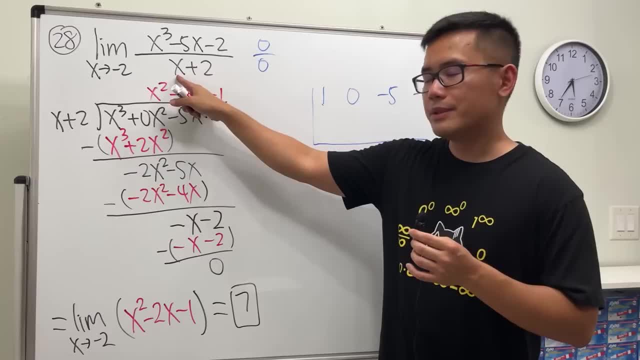 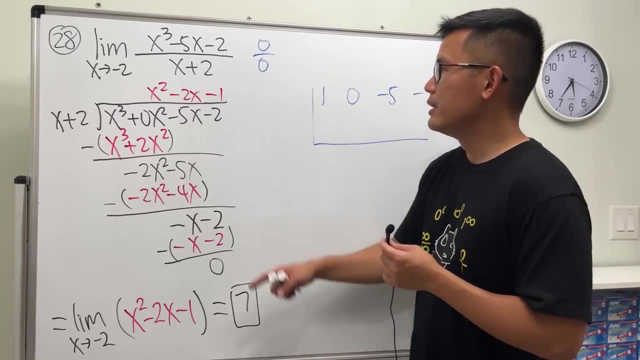 Now, here we have x plus 2. Ask yourself, how can you make this equal to 0? x has to be negative, 2, right. So we are going to do the opposite. We are going to do the opposite. We are going to do the. 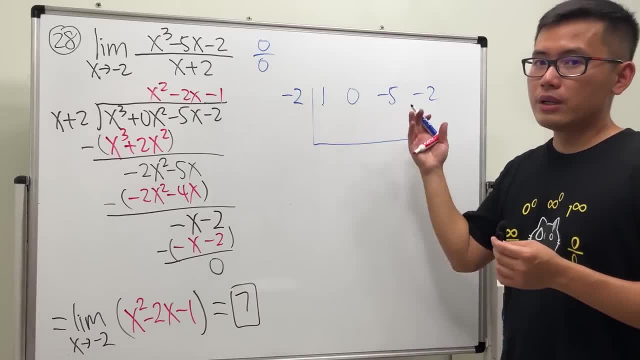 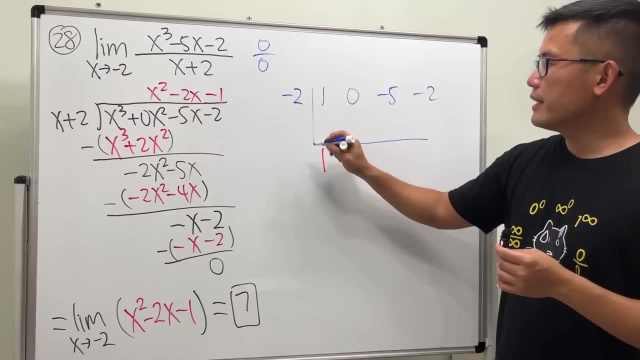 opposite of this number. so just put negative 2 right here And then for the synthetic diffusion we are going to add. Check this out. This is how we do it: First bring down the 1.. Next we do this: 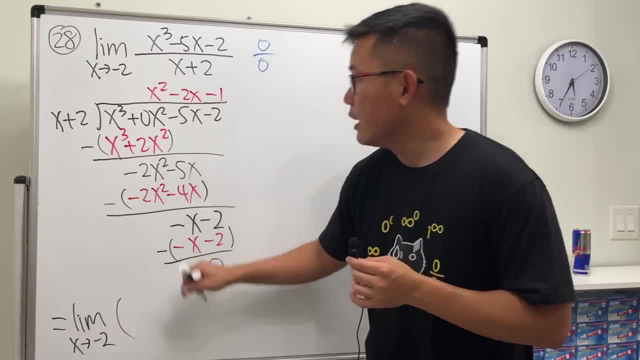 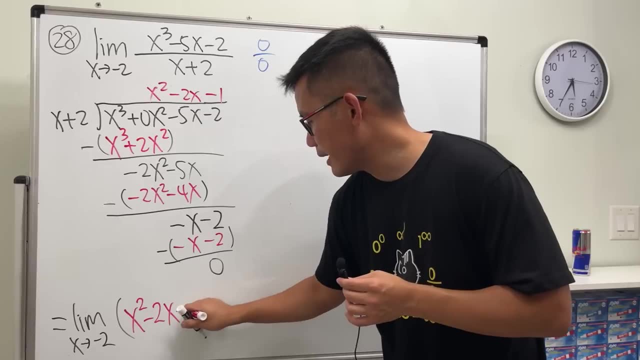 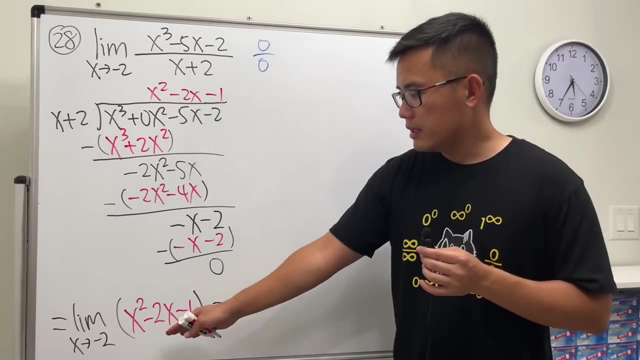 the limit as x approaching negative 2.. The whole thing reduces to that, And that's x squared minus 2x minus 1.. So what we can do at the end is just go ahead and plug in negative 2.. So negative 2 in here we get 4.. 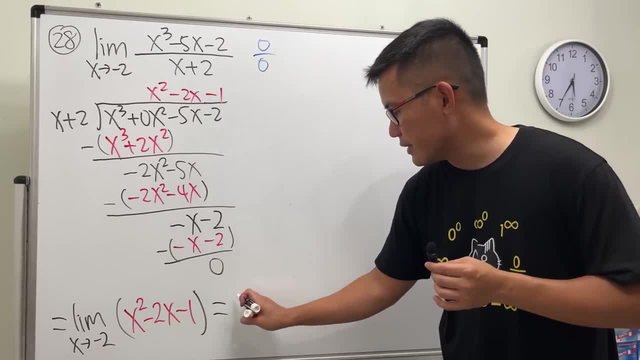 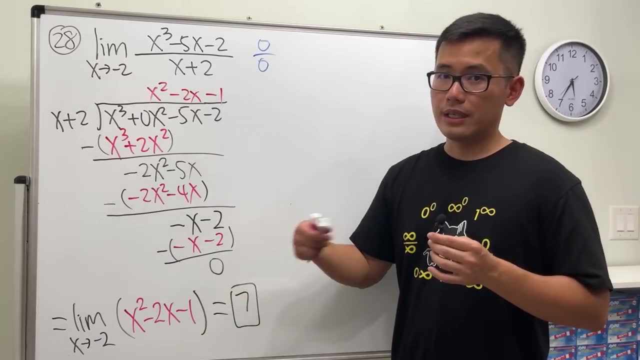 And then plus another 4 is 8. And then minus 1 is 7.. So the answer for this is 7.. All right, so last one, just you plug in, Then you evaluate. So this is another way to cancel the 0 for 0,. 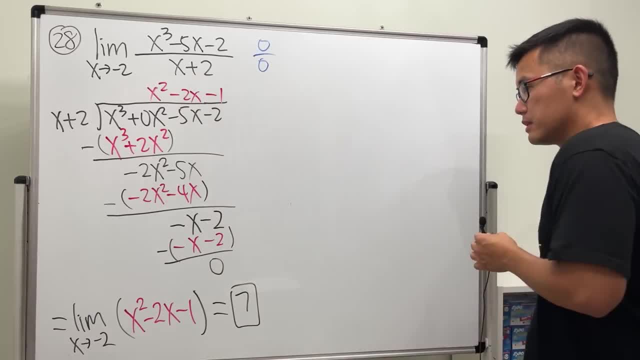 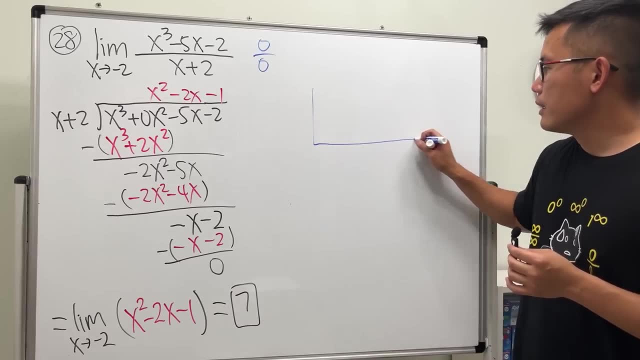 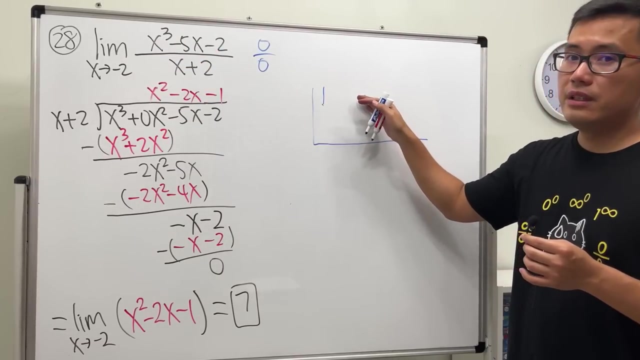 because the x minus 2 is gone. Yeah, OK, so how do we do the so-called synthetic division? then Here's the deal. Look at the coefficients, So, starting with 1, and we do not have the x squared term. 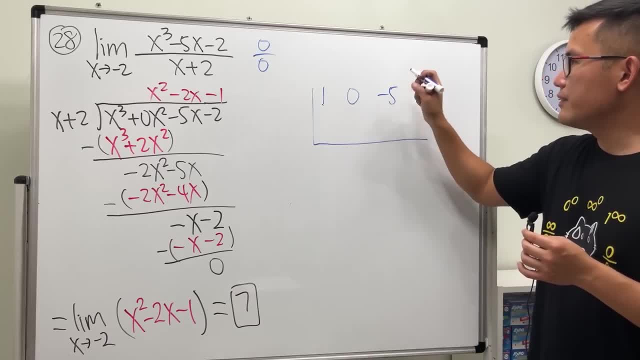 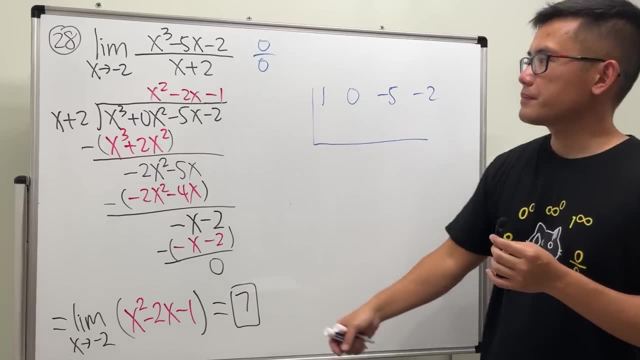 so just 0, and then minus 5, and then minus 2.. Right, So it's the same. right here: 1, 0,, negative 5,, negative 2.. Now here we have x plus 2.. 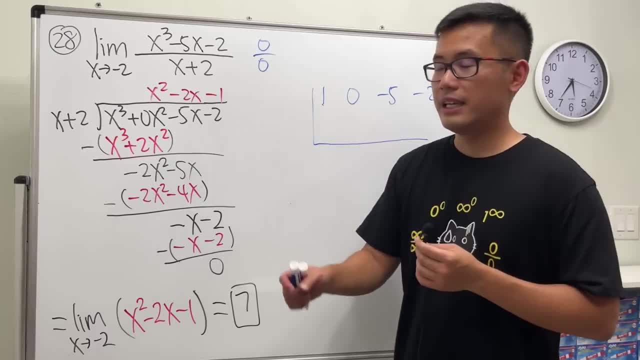 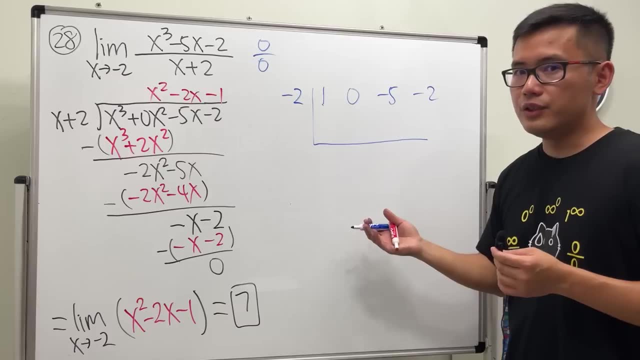 Ask yourself: how can you make this equal to 0? x has to be negative 2.. Right, So we are going to do the opposite of this number. So just put negative 2 right here, And then, for the synthetic division, we are going to add: 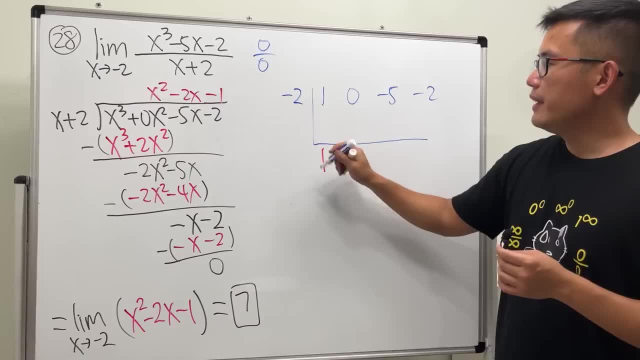 Check this out. This is how we do it: First bring down the 1.. Next we do this times that. And then- let me put it like this- We do this times that: Negative 2 times 1, we get negative 2.. 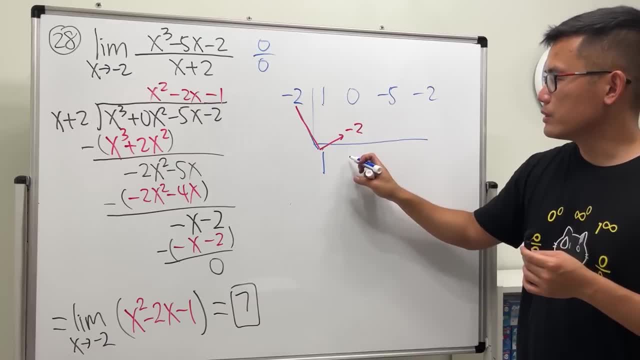 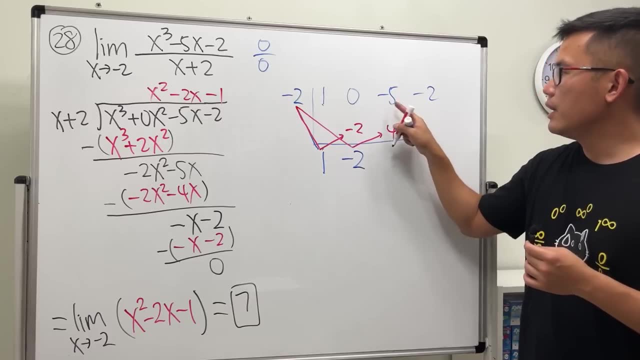 And then we are going to add, So we get 0 plus negative 2. So that will be negative 2. And then we continue: Negative 2 times negative, 2 is positive 4.. And we put it here: Negative 5 plus 4 is negative 1.. 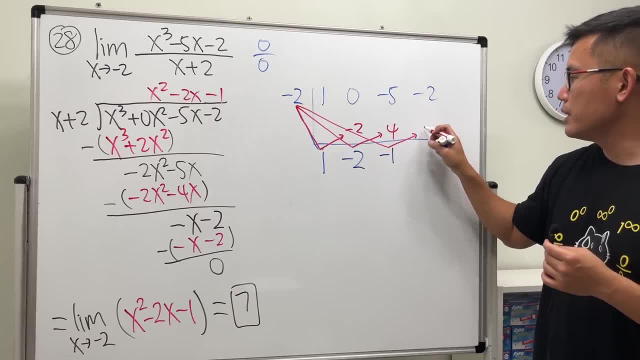 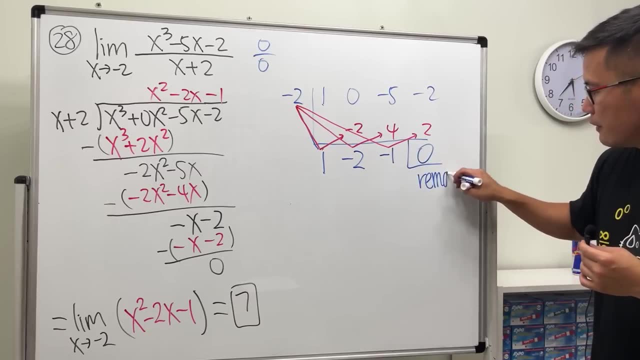 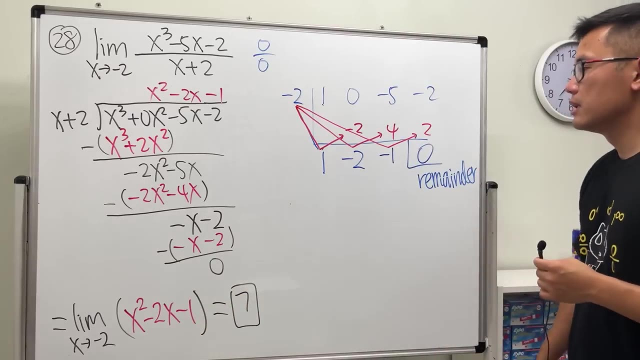 Next, this times that is positive 2.. And we put it here: Negative 2 plus 2 is 0.. This number is the remainder. Very nice. Why Remainder 0.. Just like this earlier, So like normal fraction part. 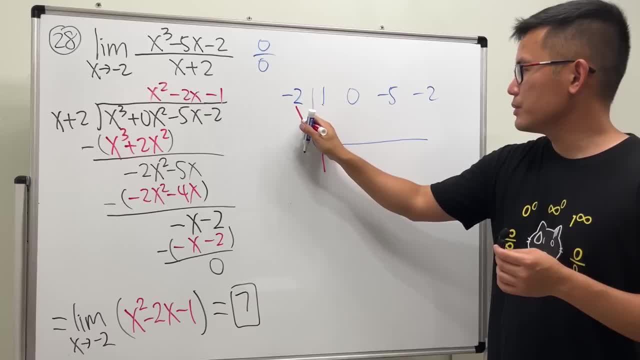 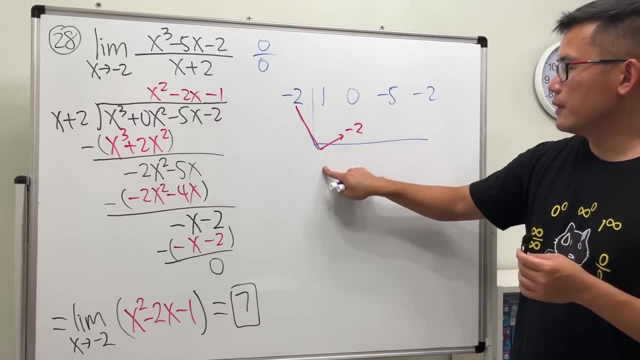 times that. and then let me put it like this: We do this: times that Negative 2 times 1, we get negative 2.. And then we are going to add so we get 0 plus negative 2, so that will be negative 2.. 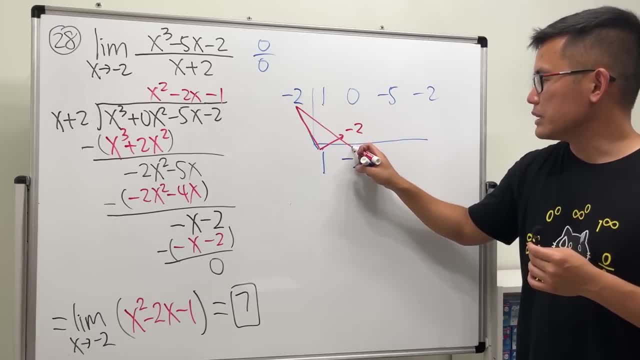 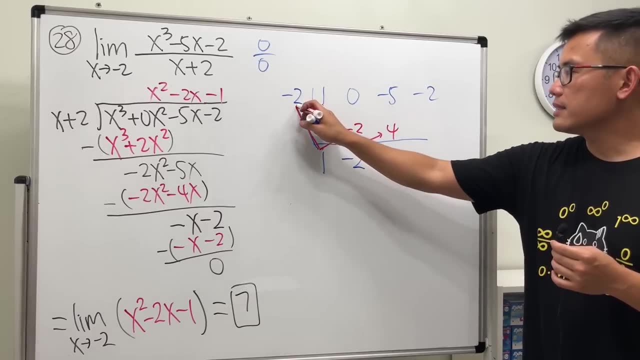 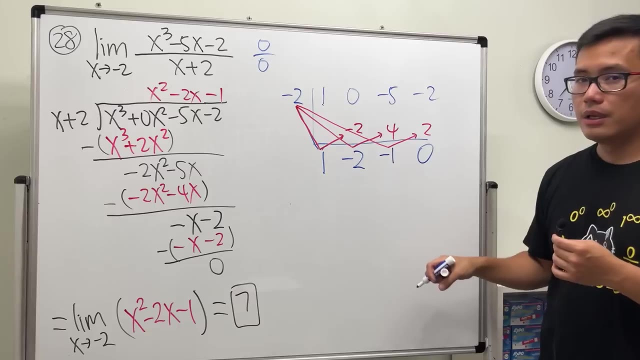 And then we continue: Negative 2 times negative 2 is positive 4, and we put it here: Negative 5 plus 4 is negative 1.. Next, this times that is positive 2, and we put it here: Negative 2 plus 2 is 0.. This number is the. 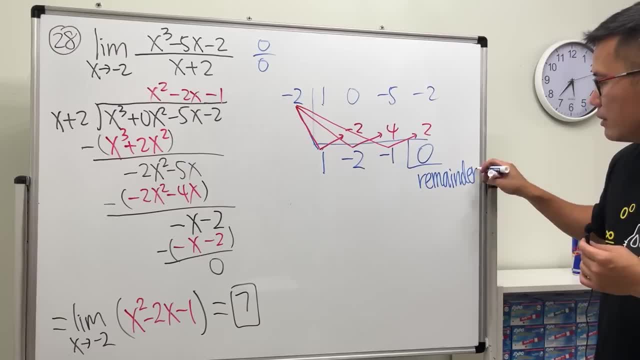 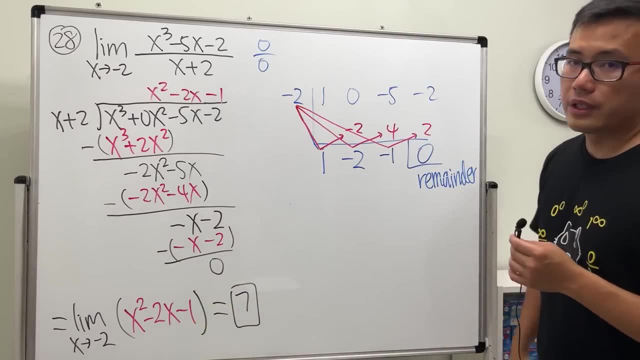 remainder Very nice. Why Remainder 0.. Just like this earlier, So like normal fraction part. So how do we read the answer from here, though? Originally this is x plus third power, right? So keep that in mind: x plus third power and x. 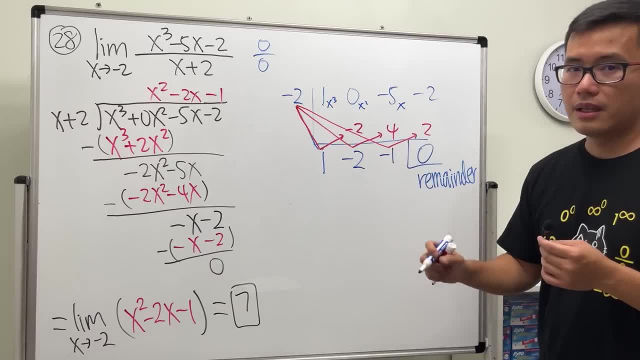 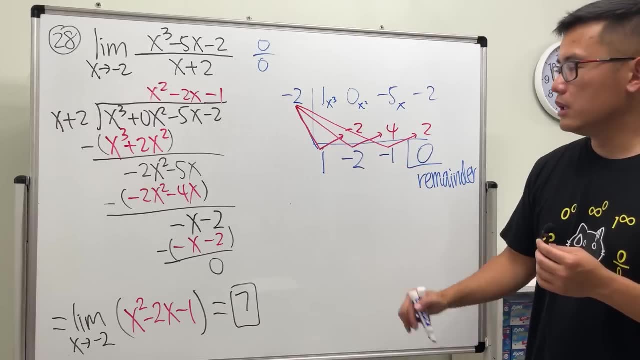 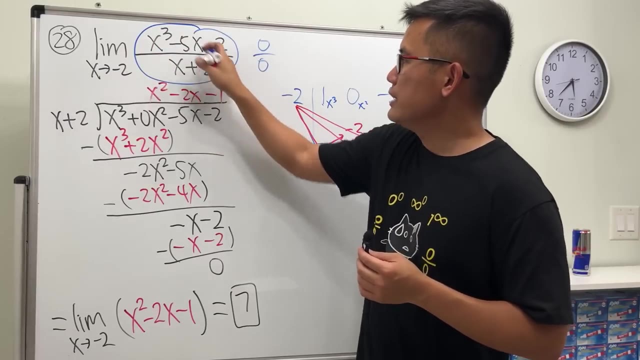 squared. You don't have to write it down for that. Just keep that in mind When we do the synthetic diffusion. these are the coefficients for our answers, and the power goes down by 1.. So we have the x squared x and also no x. So, as you can see, this part becomes x squared minus 2x. 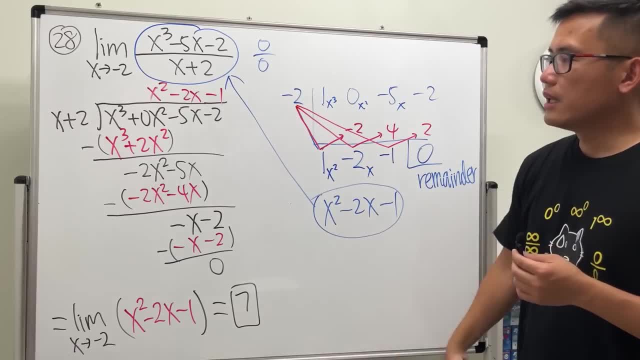 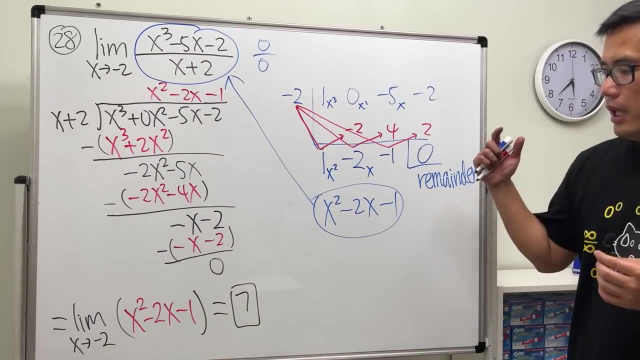 minus 1. Stop, And of course, once you put this back here, we do the same thing, And then you can compute it and we get 7.. All right, so again just a way to kind of get rid of the rational expression case. 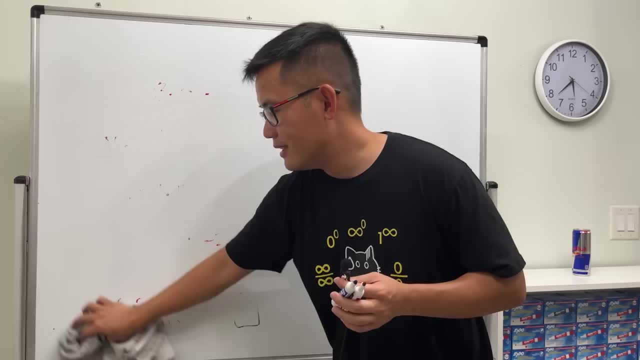 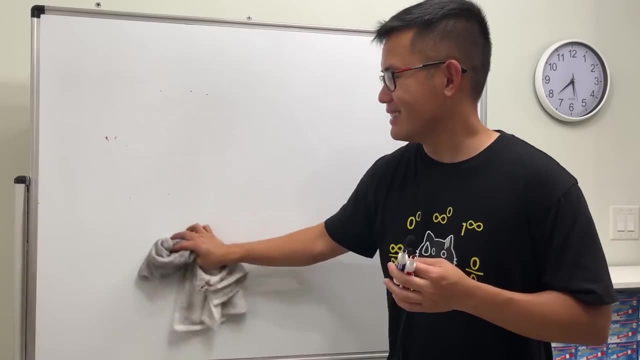 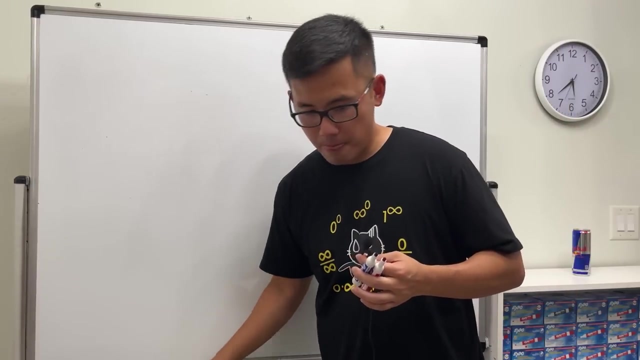 You know the hard questions are at the end, Absolutely. I don't know if you forgot, but we have this epsilon delta definition of the limit and the Riemann sound integrals- pretty much the definition of integrals, almost like that. 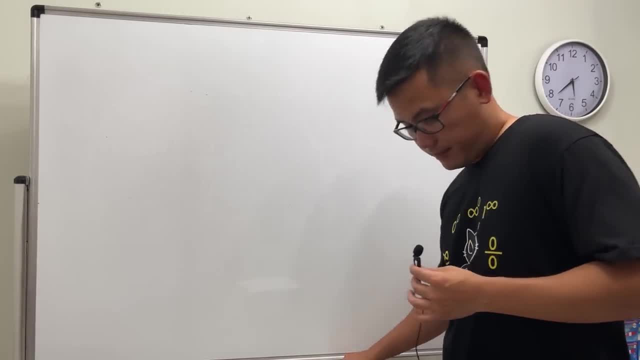 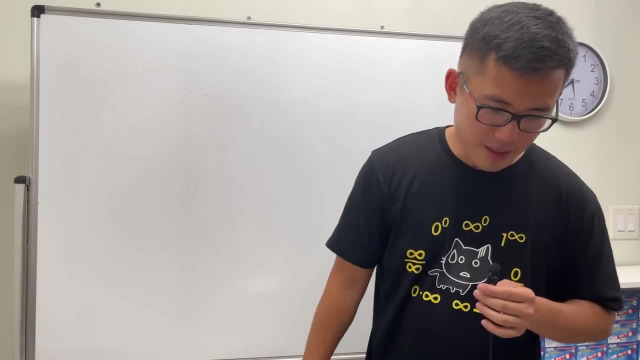 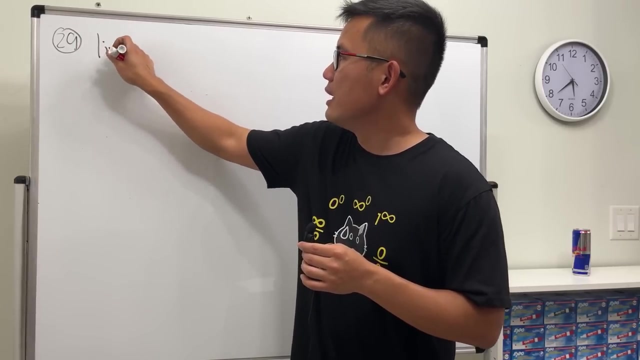 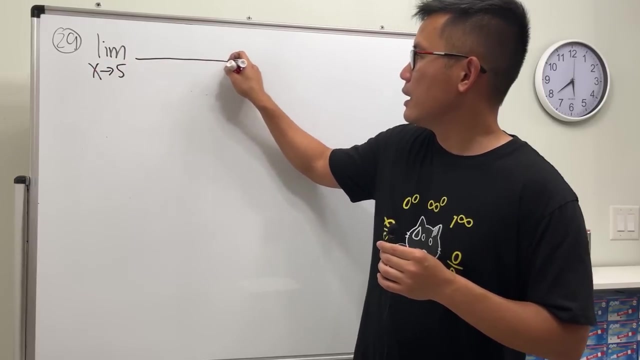 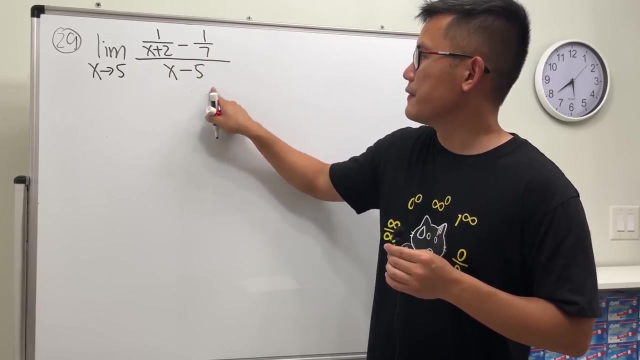 Yeah, Okay, Oh, we'll also be doing the derivative, the definition of derivative, though It's coming. Yeah, By the way, couple more to go Number 25.. Here we have the limit, and then we have x approaching 5, 1 over x plus 2 minus 1 over 7, and x minus 5.. 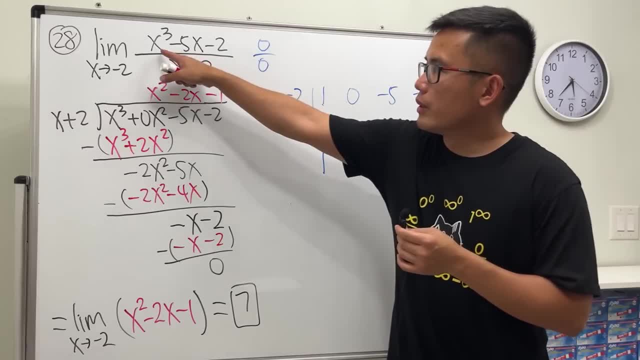 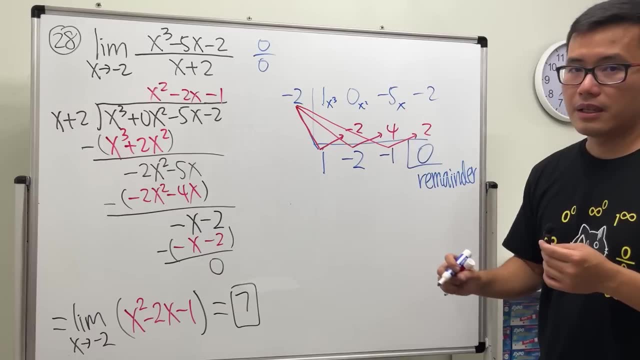 So how do we read the answer from here, though? Originally this is x plus 3rd power, So keep that in mind: x plus 3rd power and x squared. You don't have to write it down for that, Just keep that in mind. 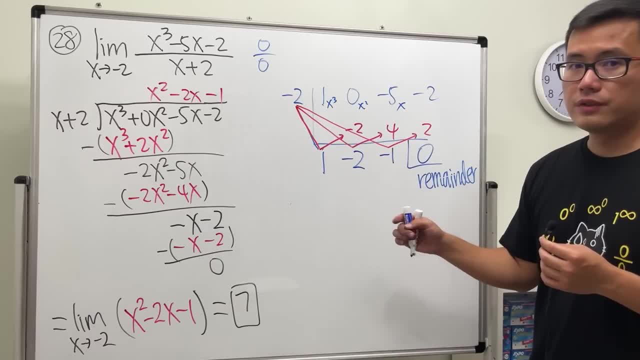 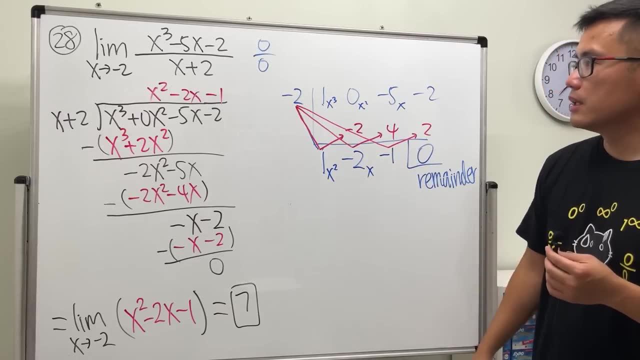 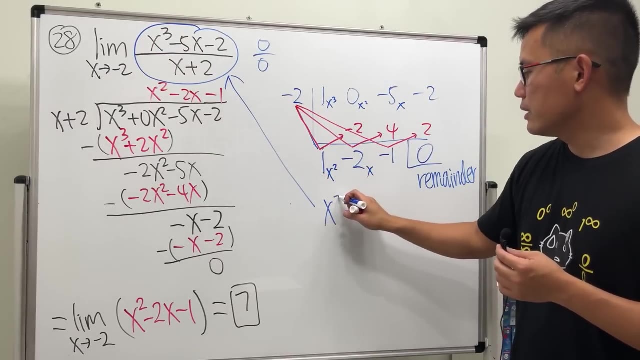 When we do the synthetic division. these are the coefficients for our answers, And the power goes down by 1.. So we have the x squared x and also no x. So, as you can see, this part becomes x squared minus 2x minus 1.. 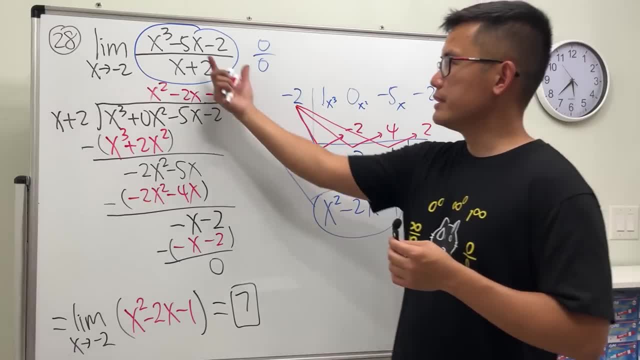 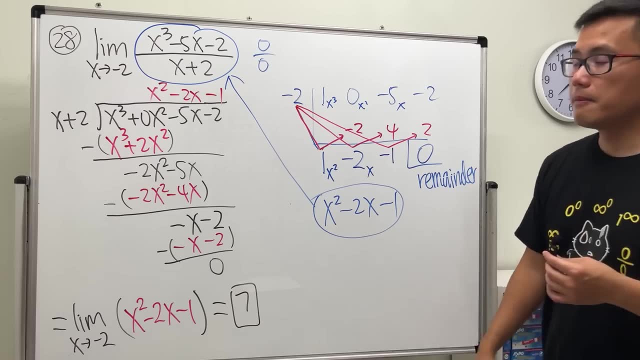 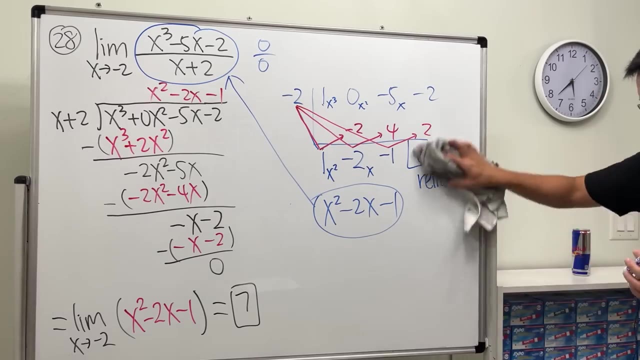 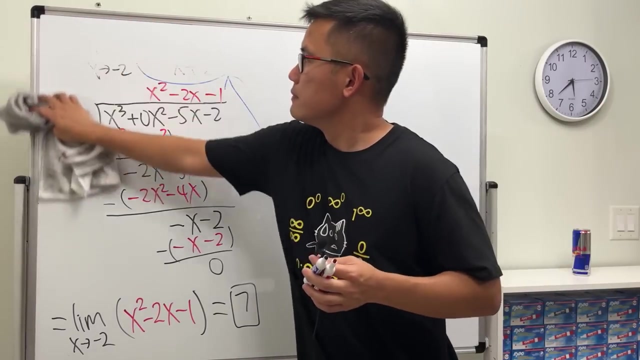 So it's that, And of course, once you put it back here, we do the same thing, And then you can compute it And we get 7.. All right, So again just a way to kind of get rid of the rational expression case. 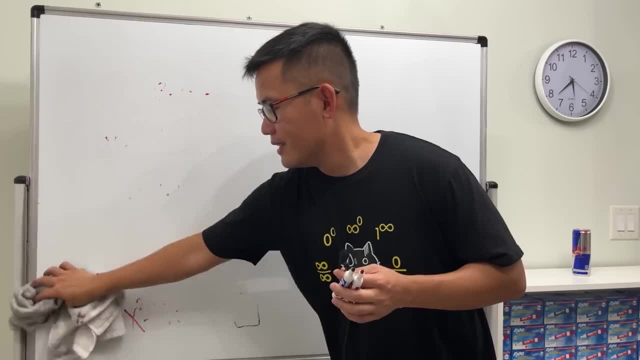 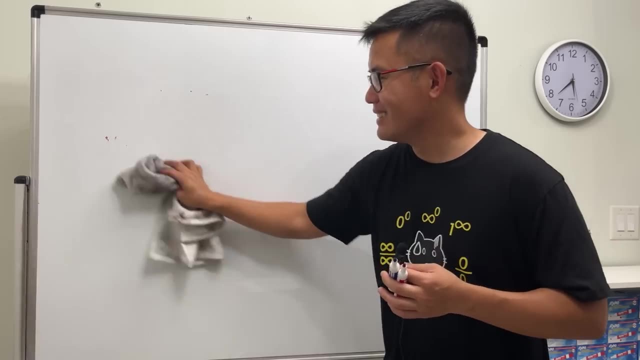 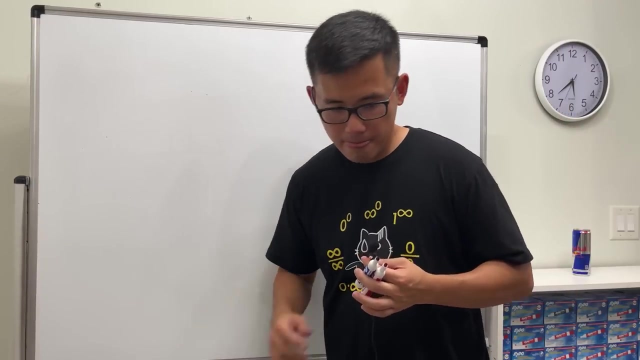 You know, the hard questions are at the end: Epsilon, delta, definitions of the limit and also the Riemann sum Integrals, pretty much Definition of integral, technically Almost like that. Yeah, Wee, OK, Oh, we will also be doing the derivative. 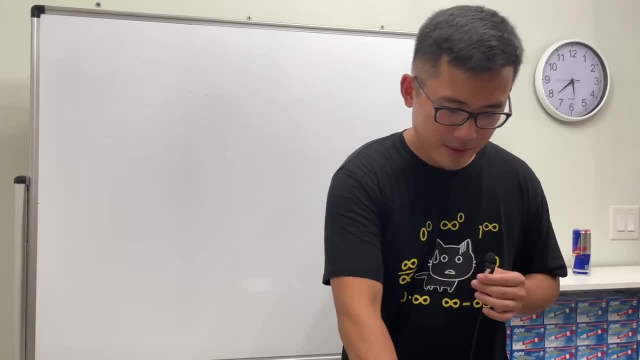 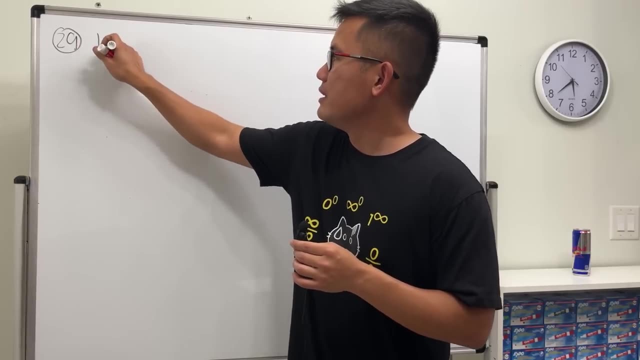 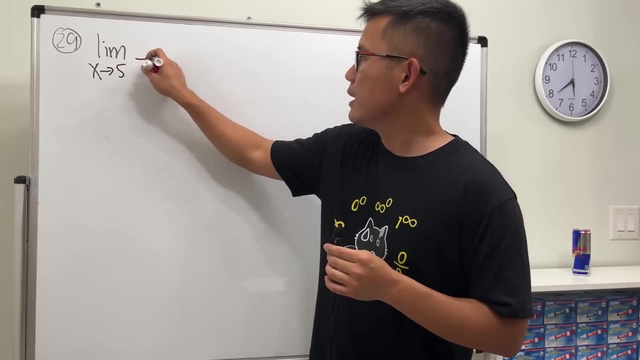 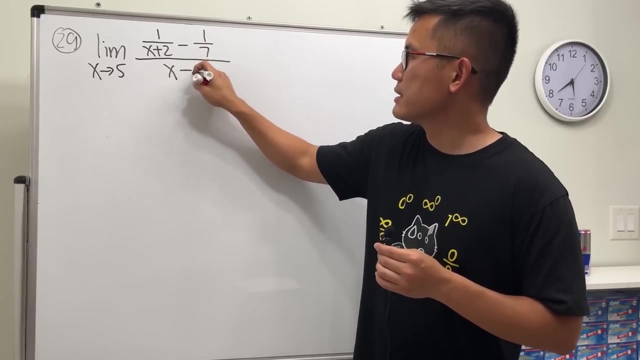 The definition of derivative, though It's coming. Yeah, By the way. couple more to go Number 29.. Here we have the limit, And then we have x approaching 5.. All right, So we have 1 over x plus 2 minus 1 over 7 and x minus 5.. 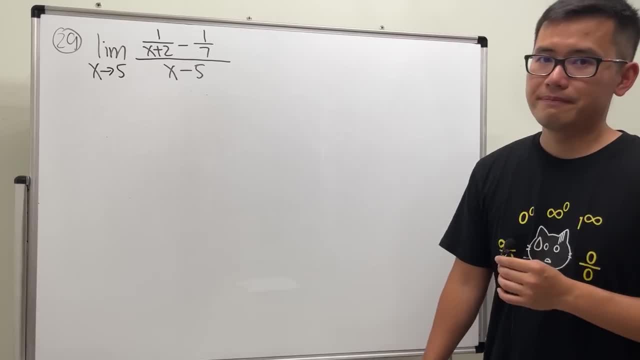 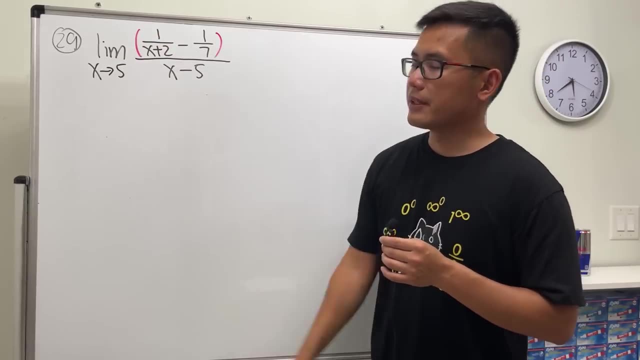 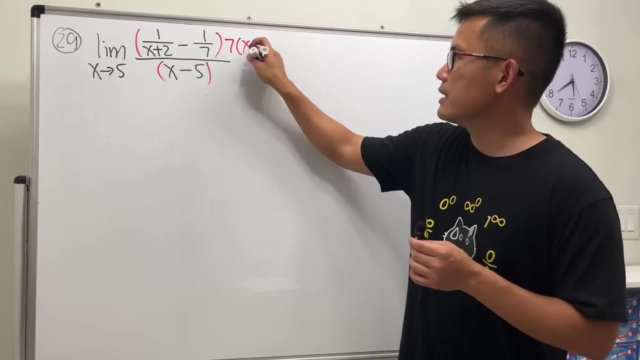 Here we have a complex fraction, So how do we simplify this? The key is that we don't like complex fractions, So I would recommend you guys to multiply the top and bottom by this and that just like the common denominator. So I'll put it at 7 times x plus 2.. 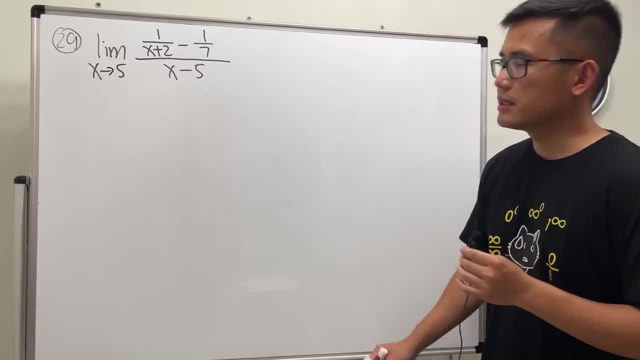 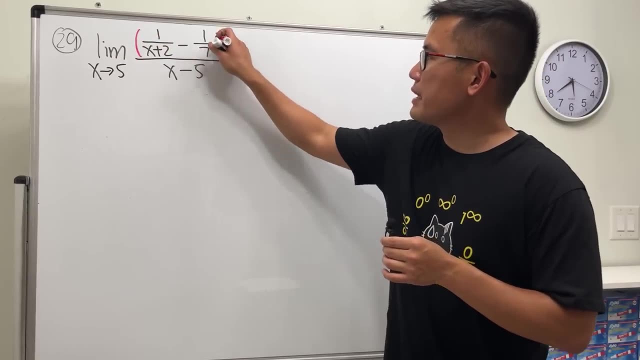 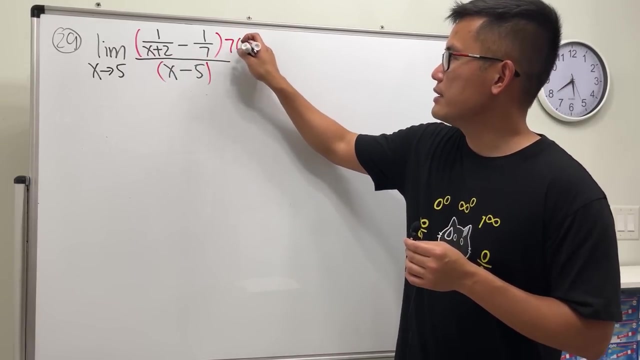 Here we have a complex fraction, so how do we simplify this? The key is that we don't like complex fractions, So I would recommend you guys to multiply the top and bottom by this and that just like the common denominator. So I would put it as 7 times x plus 2, likewise the bottom. 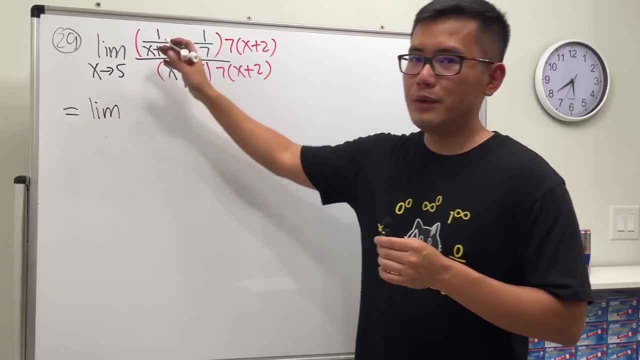 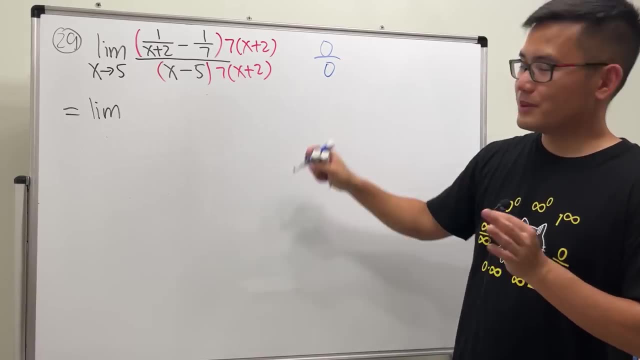 Check this out. This is going to give us the limit. Oh, by the way, it would be 0 over 0, I forgot to say that 1 over 7 minus 1 over 7, and then 5 minus 5 is 0 over 0.. 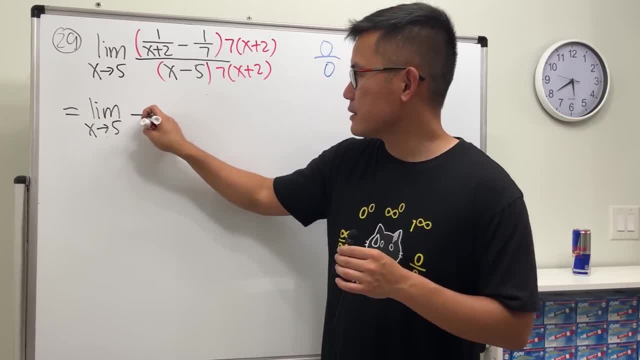 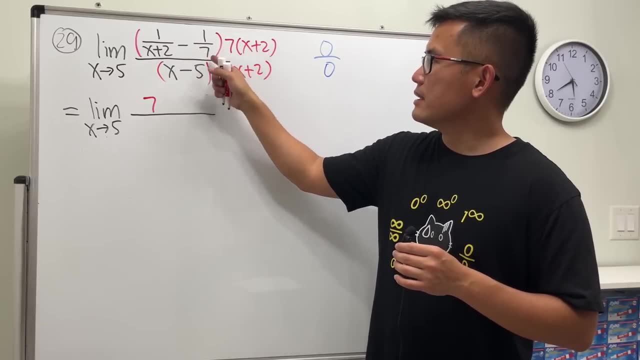 Anyway, limit as x approaching 5. Take this multiply by that, we will just have the 7 left. Then take this multiply by that, the 7 will cancel. so we have this minus And then we have the x plus 2.. 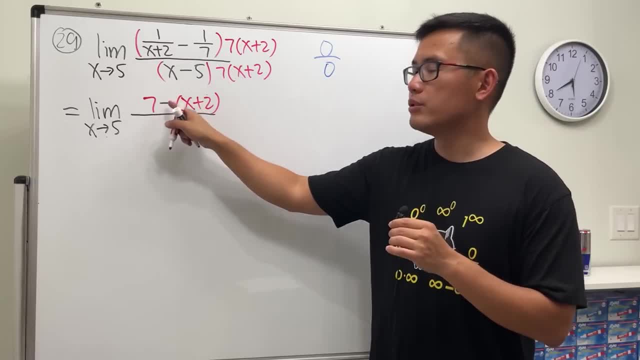 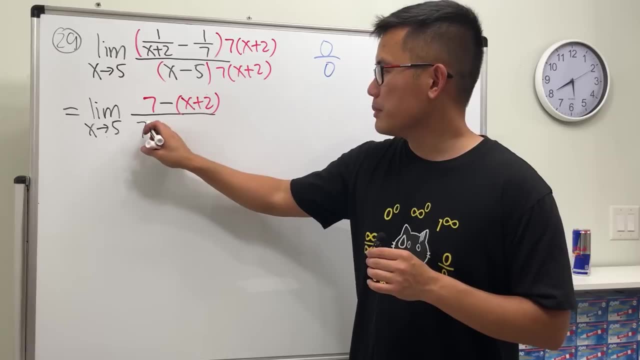 But be sure to put parentheses around it, because we will have to distribute the negative in a second On the bottom. I'm just going to rewrite it Here we have the 7 goes first. Do not multiply out anything. So 7, and then x minus 5, and then x plus 2.. 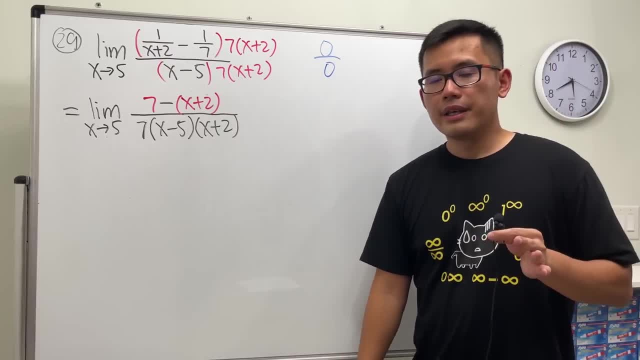 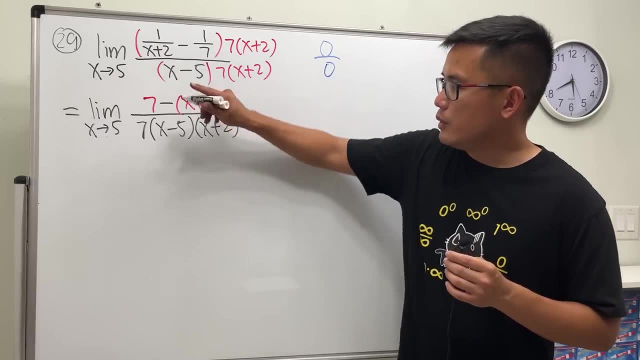 Okay, here's a very common mistake. A lot of students, once they get to here, they see the x plus 2, x plus 2, then in parentheses, they will just cancel it. This is wrong. The reason is because we must fix the top first, the world of operations. 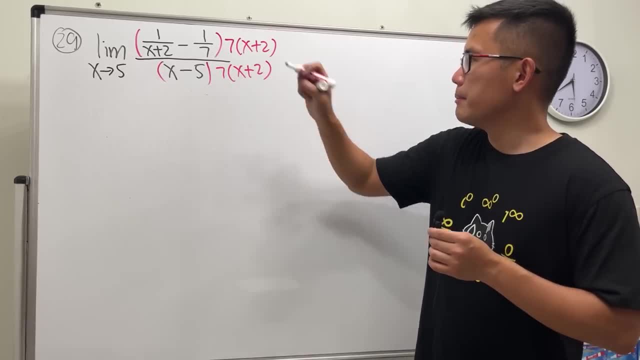 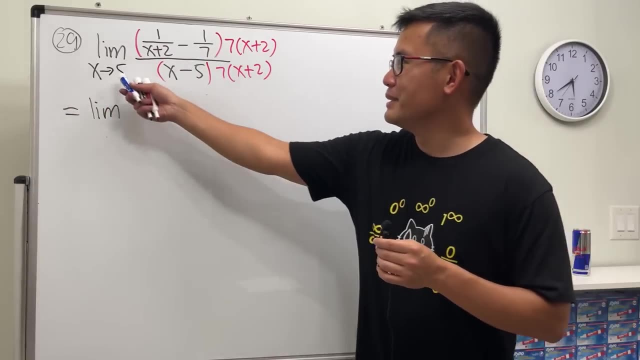 Likewise the bottom. Check this out. This is going to give us the limit. Oh, by the way, it would be 0 over 0.. I forgot to say that 1 over 7 minus 1 over 7.. 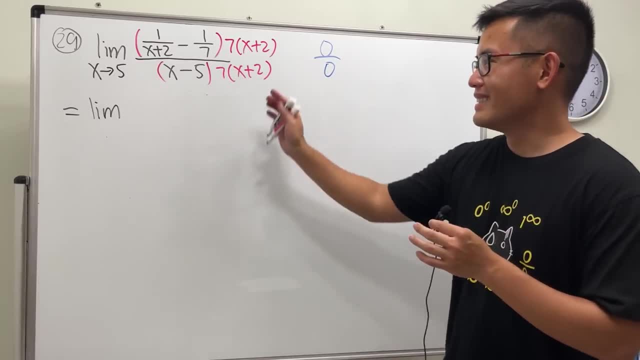 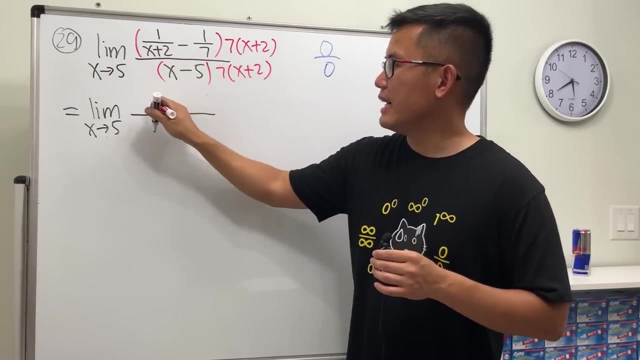 And then 5 minus 5 is 0 over 0. Anyway, Limit as x approaching 5.. Take this, multiply by that, We will just have the 7 left. Then take this, multiply by that, The 7 will cancel. 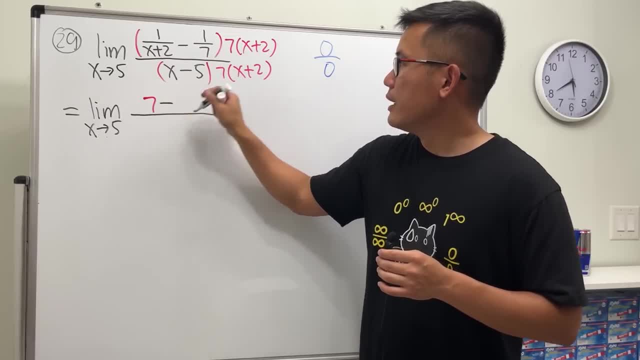 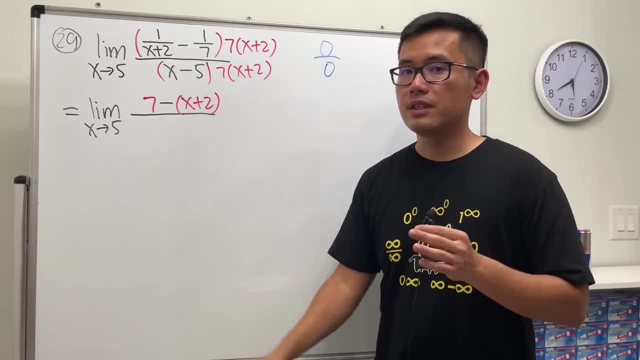 So we have this minus And then we have the x plus 2. But be sure to put parentheses around it, because we will have to distribute the negative in a second On the bottom. I'm just going to write it Here. we have the 7 goes first. 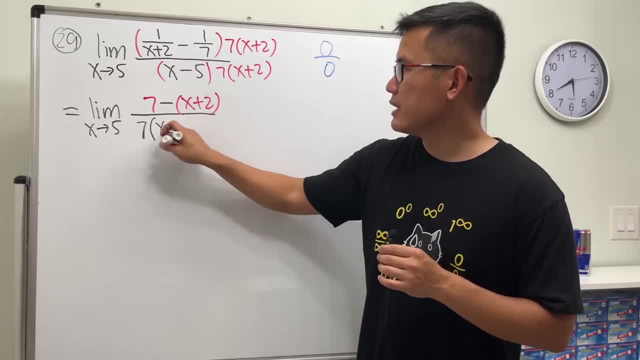 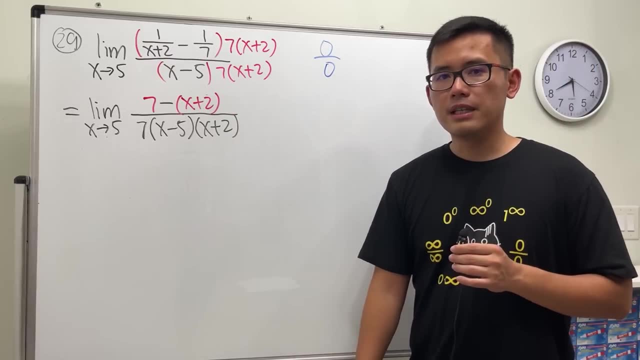 Do not multiply out anything. So 7 and then x minus 5 and then x plus 2.. OK, Here's a very common mistake. A lot of students, once they get to here, they see the x plus 2, x plus 2.. 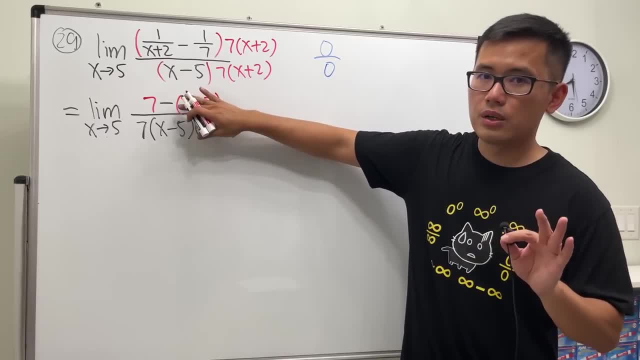 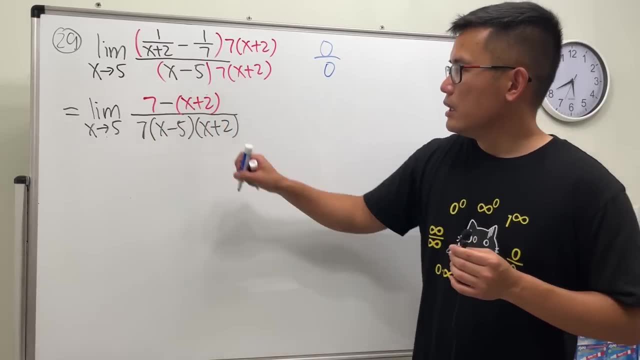 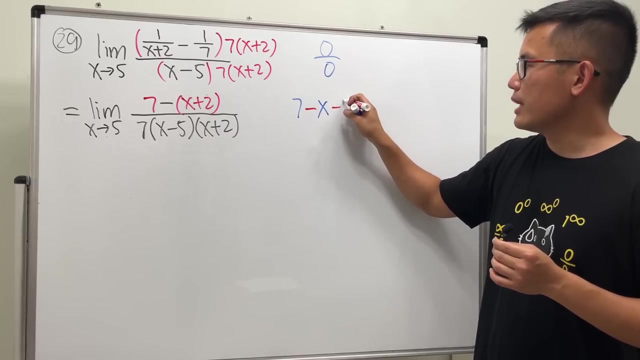 Then in parentheses, they will just cancel it. This is wrong. The reason is because we must fix the top first, The world of operations. So let's see For the top. we will just get 7 and then distribute. We get negative x and then minus 2, right. 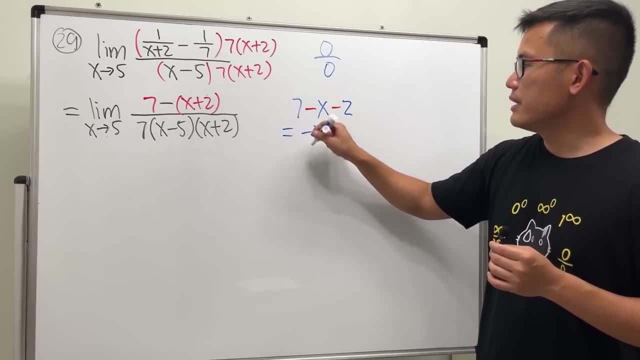 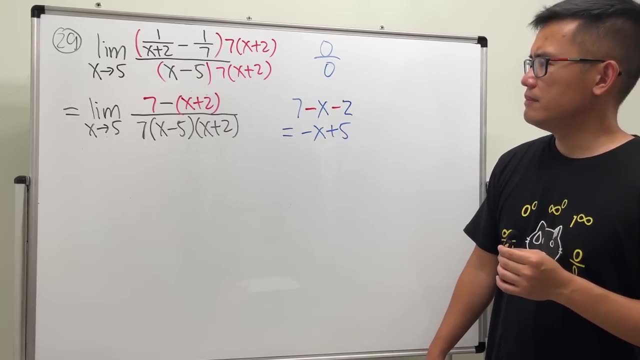 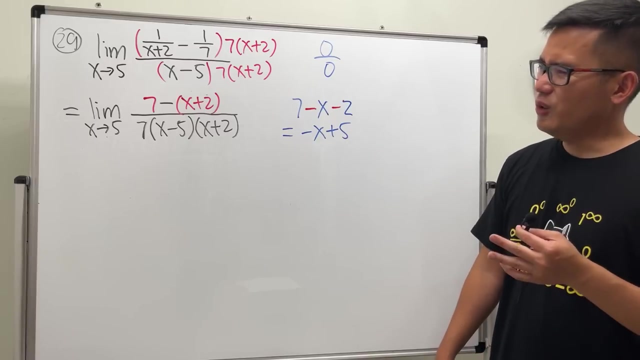 So, all in all, we just get negative x, and then this is plus 5.. Yeah, Hmm, Hey, This is x minus 5.. This is negative x plus 5.. They are almost the same. Don't worry, Let's factor out an x. 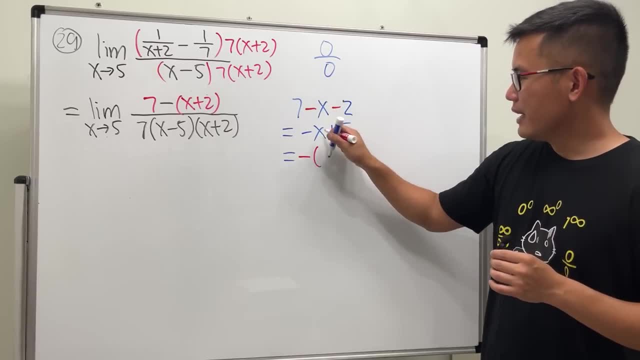 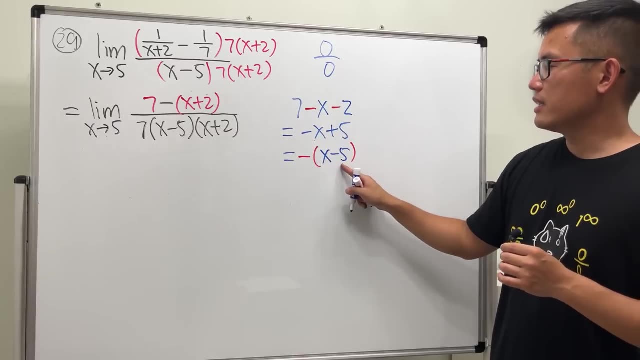 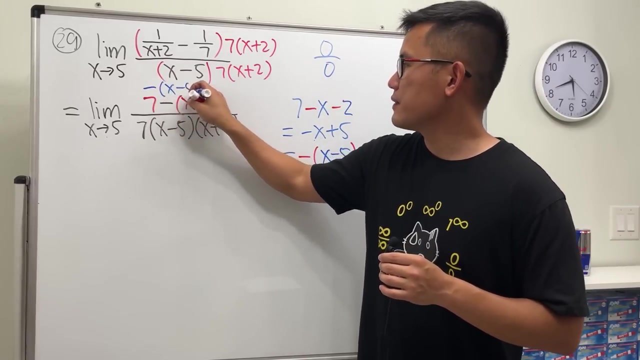 Sorry, Let's factor out a negative. So let's put a negative like so, And then we can change this to be x and then minus 5.. Check: Negative, x, negative, negative. We get the positive. So the top right here is negative and then x minus 5.. 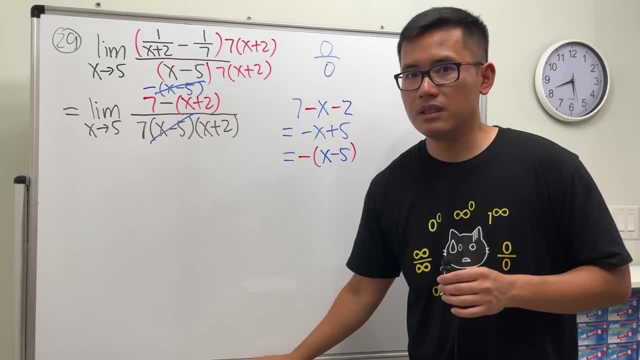 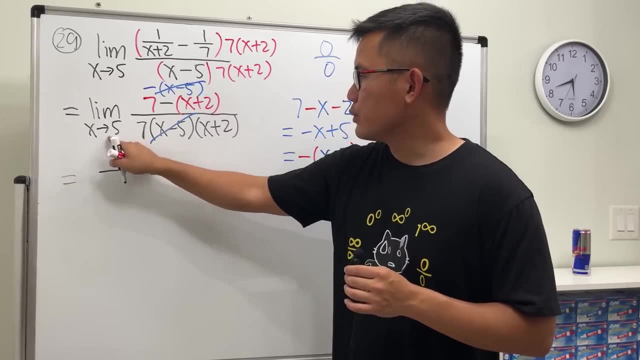 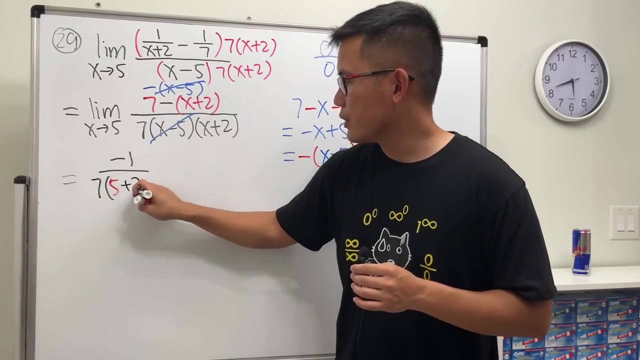 Now cancel, cancel. This is the right way to do it. On the top, we have negative 1.. On the bottom, we're plugging the 5 here. So we see, here we have the 7 times 5 plus 2, which is just 7.. 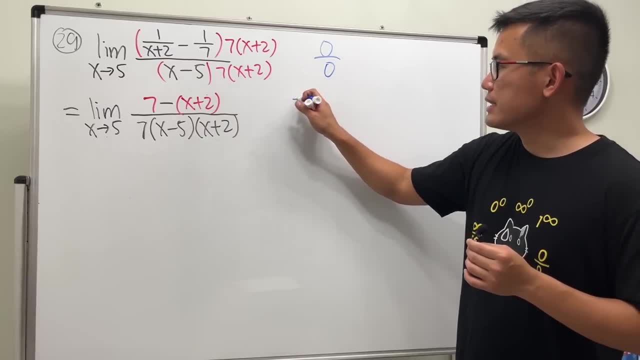 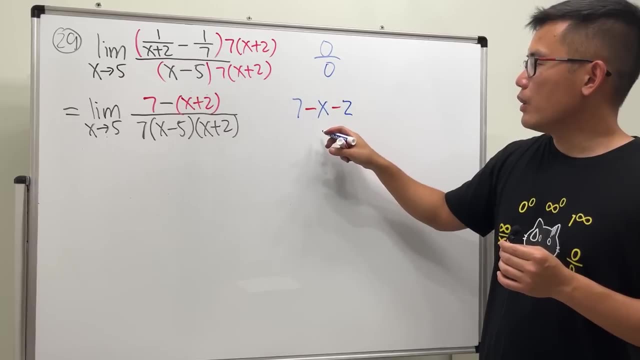 So let's see For the top, we will just get 7, and then distribute, we get negative x and then minus 2, right? So all in all, we just get Negative x and then this is plus 5.. 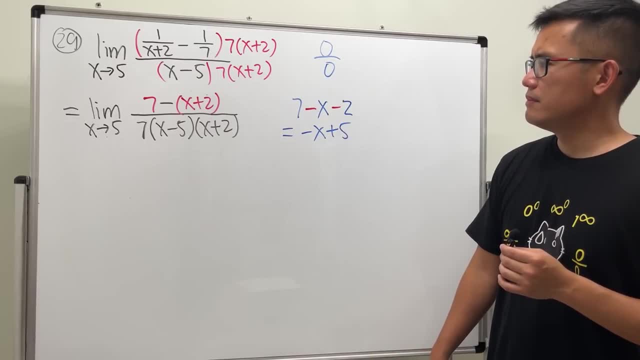 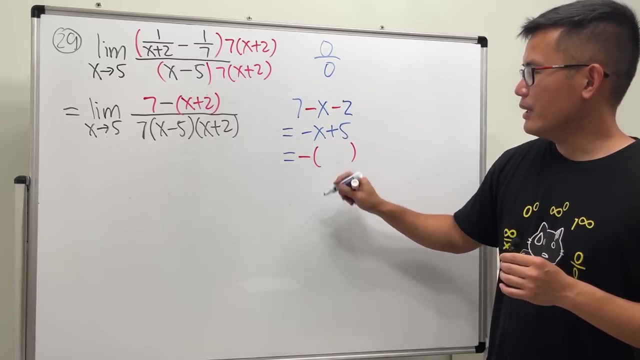 Yeah, Hey, this is x minus 5,, this is negative x plus 5.. They're almost the same, Don't worry. Let's factor out an x. So let's factor out a negative. So let's put a negative like so. 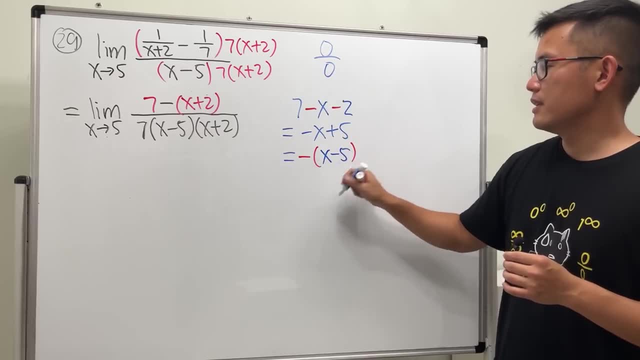 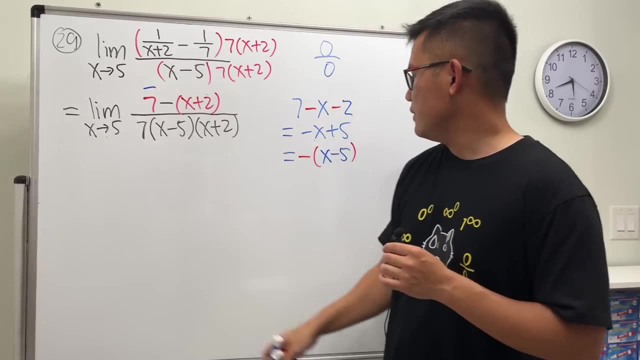 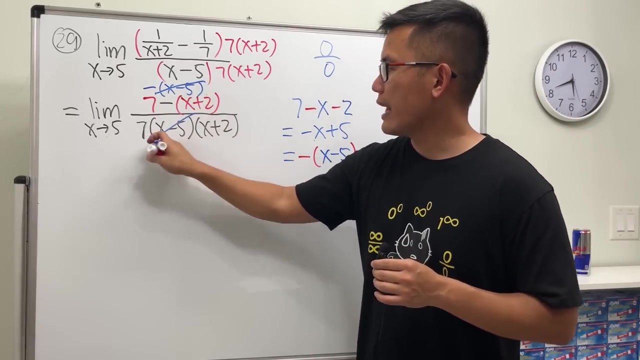 And then we can change this to be x and then minus 5.. Check Negative x, Negative Negative: we get the positive. So the top right here is negative and then x minus 5.. Now cancel. cancel. 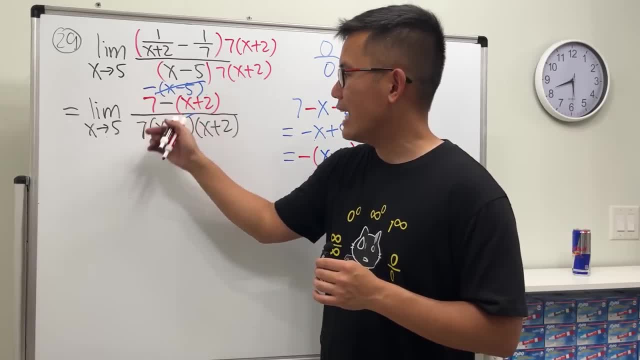 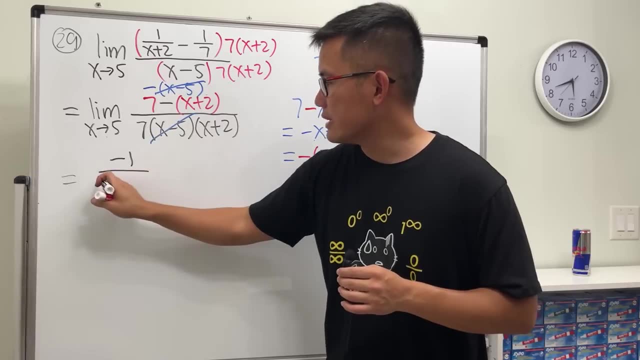 This is the right way to do it. On the top, we have negative 1.. On the bottom, we're plugging the 5 here. So we see, here we have the 7 times 5 plus 2, which is just 7.. 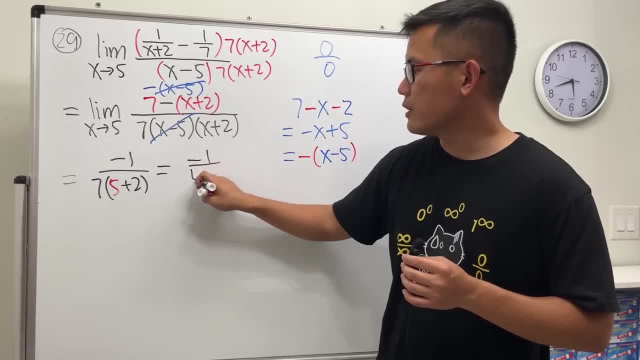 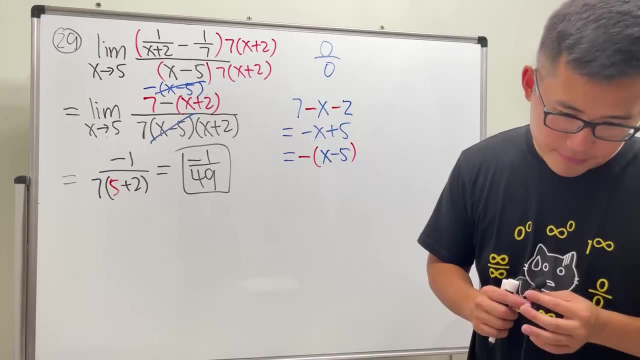 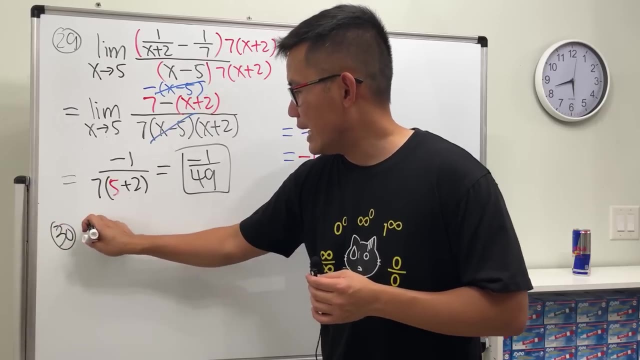 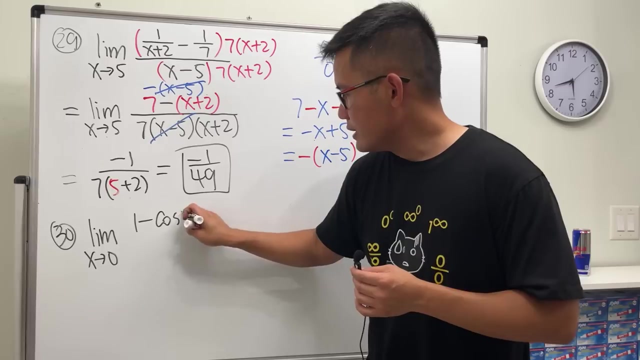 7 times 7 is 49. So we get negative 1 over 49. Okay, All right. Number 30. Here we have the limit as x approaching 0. And then we have 1 minus cosine x over sine x. 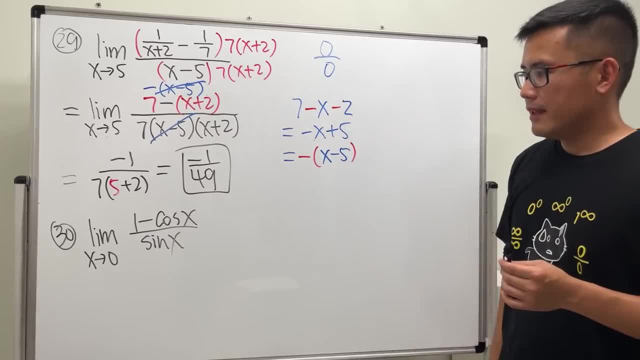 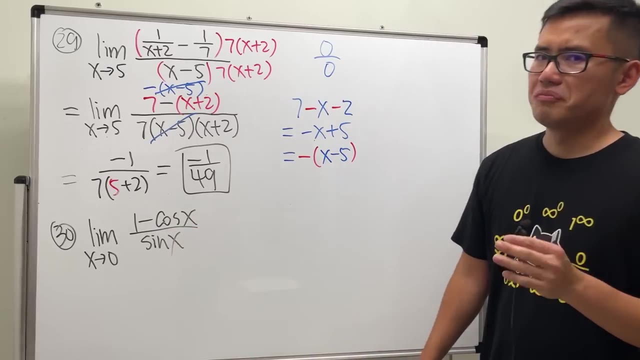 What? How do we even do this? Wow, How do we factor it? No, we are not supposed to factor it. Check this out: 1 minus cosine squared. Don't know too much about it. However, we do know that. 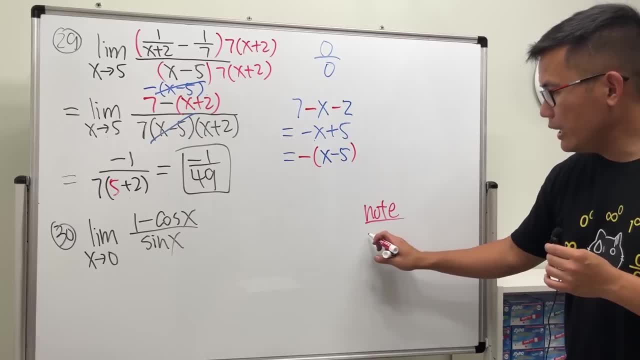 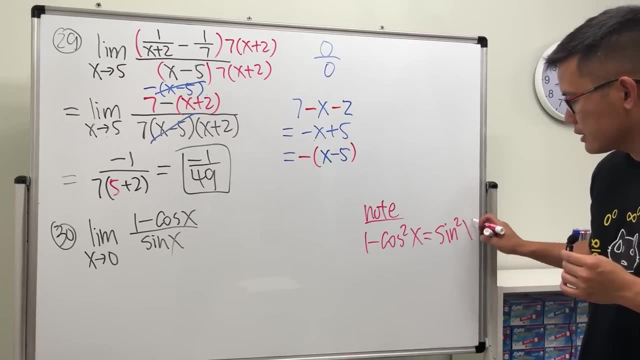 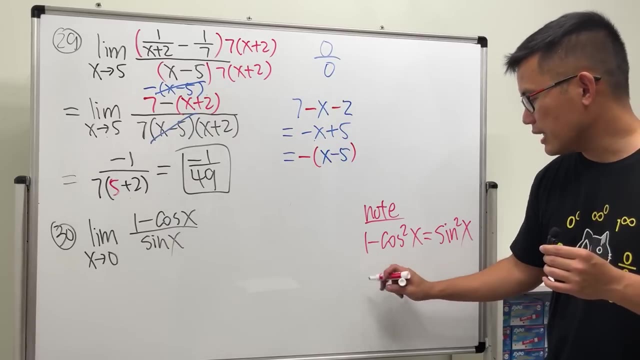 Let me just put it down right here: If we have 1 minus cosine squared x, this right here is nicely equal to what Sine squared x. Yeah, Yeah. So how can we go from here to here? Well, this is precisely 1 minus cosine x times 1 plus cosine x. 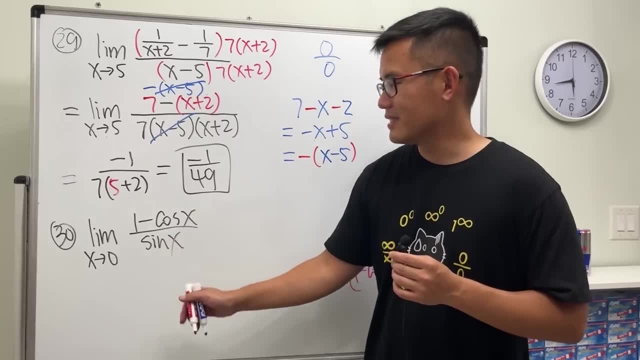 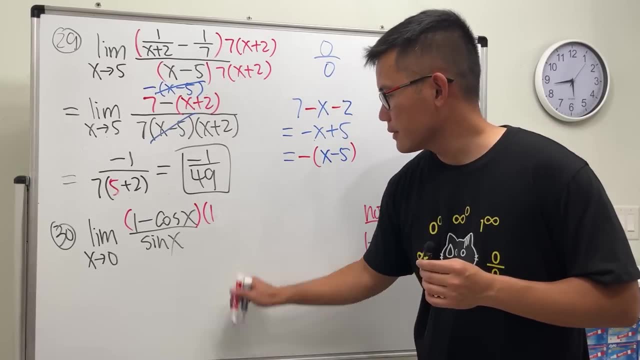 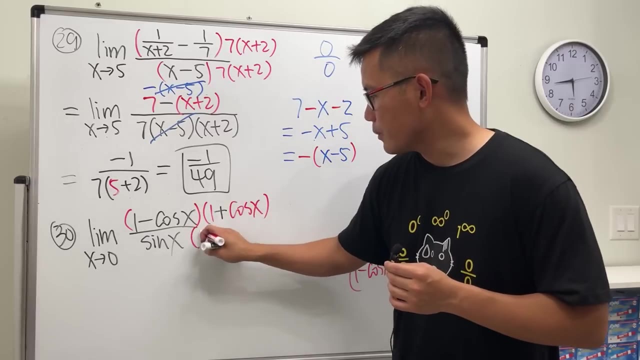 Yeah. So let's again just do the count, you get business. Take the top, multiply by 1 plus cosine x, And then, of course, we will do the same on the bottom: 1 plus cosine x. All right, 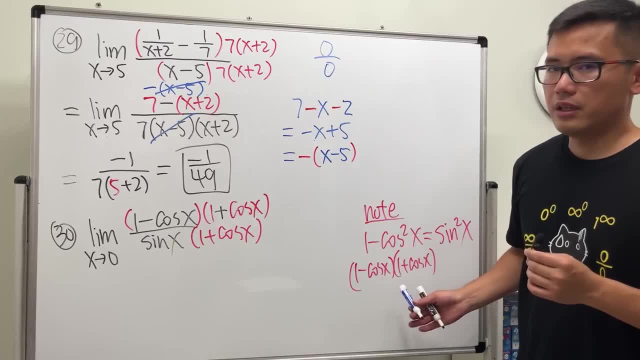 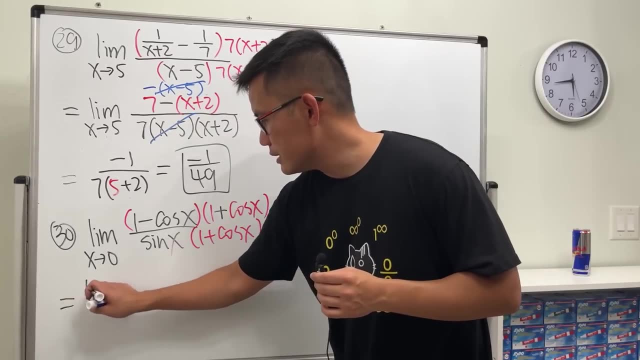 And then, per our discussion here, when we do this times, that we will just get sine squared x. That's very nice. So this right here is the limit as x approaching 0.. All in all, the top is sine squared x. 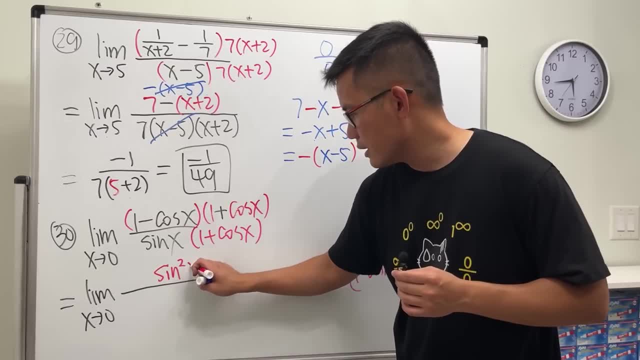 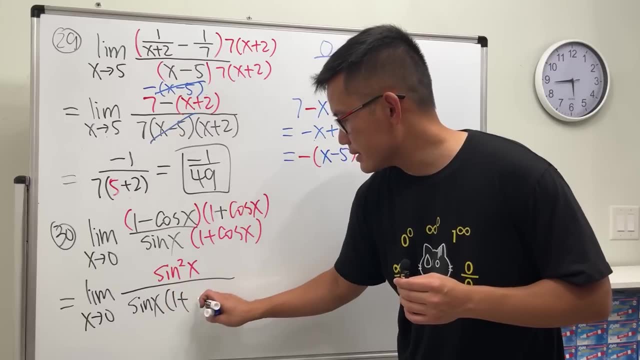 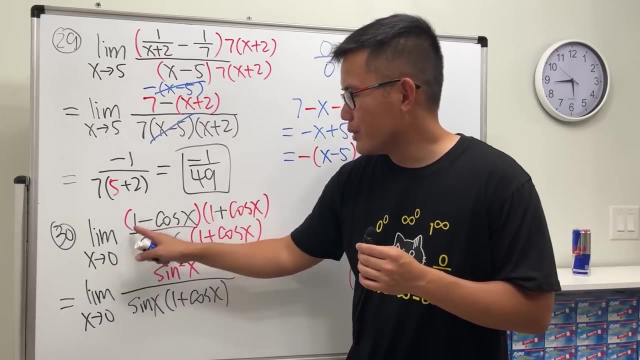 I'm just going to put that down in red. And then we have what? Here we have the sine x, And then here we have the 1 plus cosine x. Oh, by the way, I forgot to mention. The reason that we have to do this is because when we put 0 into cosine, x is 1, 1 minus. 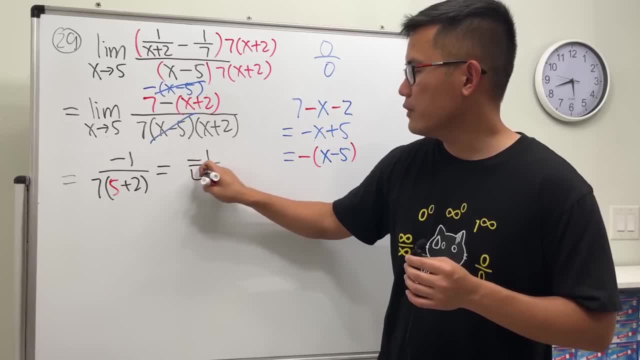 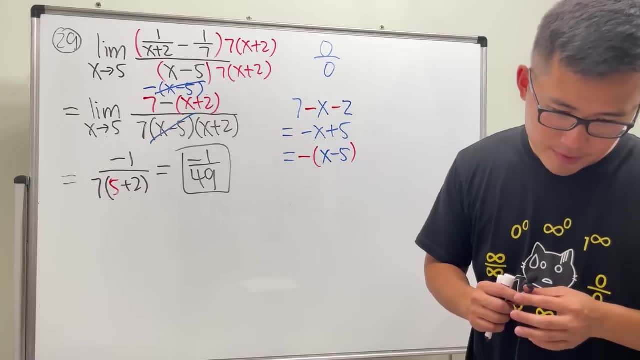 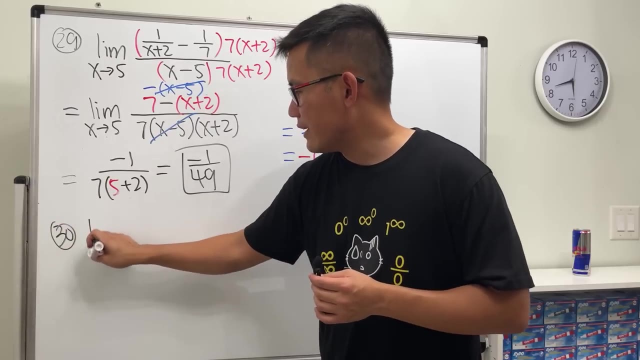 7 times 7 is 49. Altogether negative, 1 over 49.. All right, All right. Number 30. Here we have the limit as x approaching 0. And then we have 1 minus cosine x over sine x. 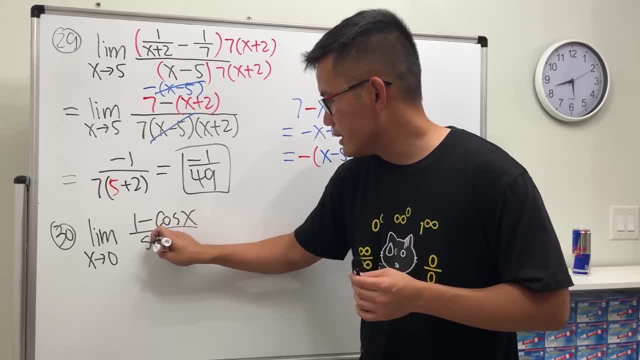 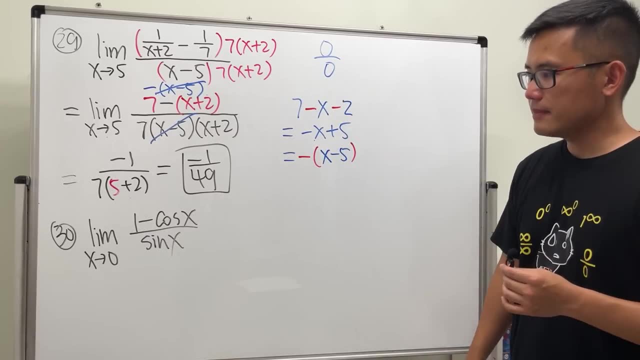 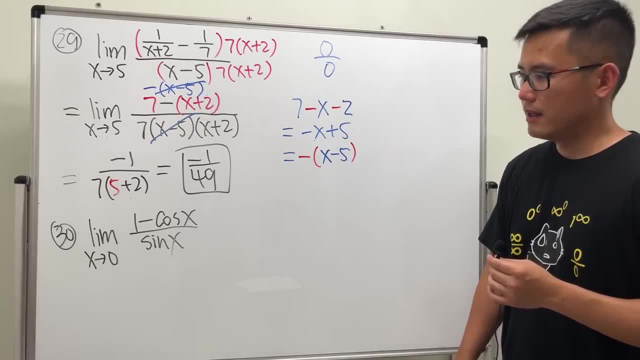 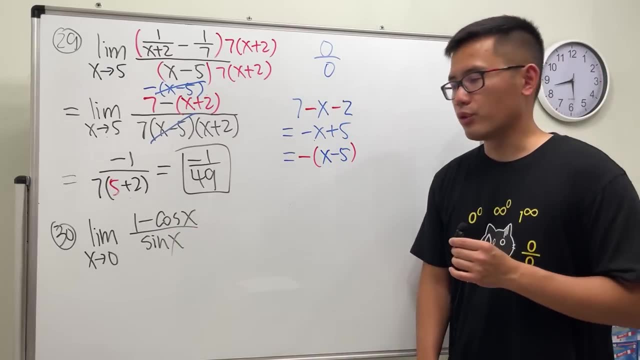 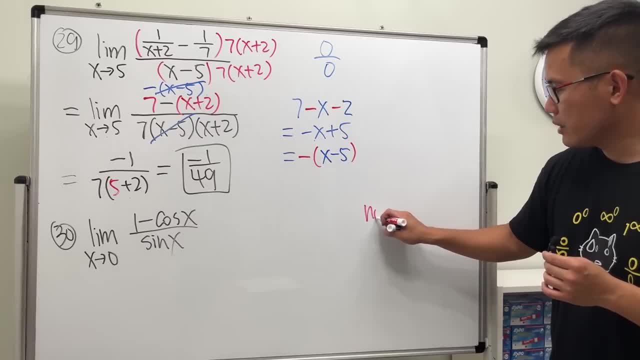 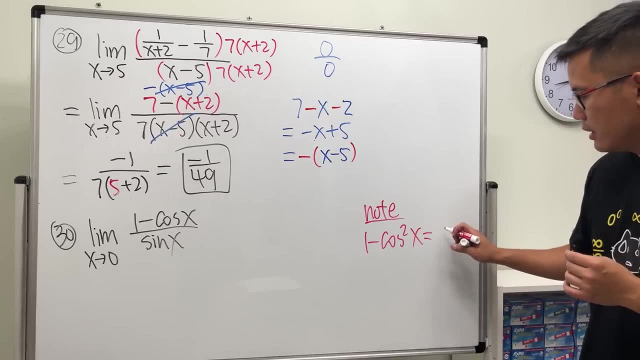 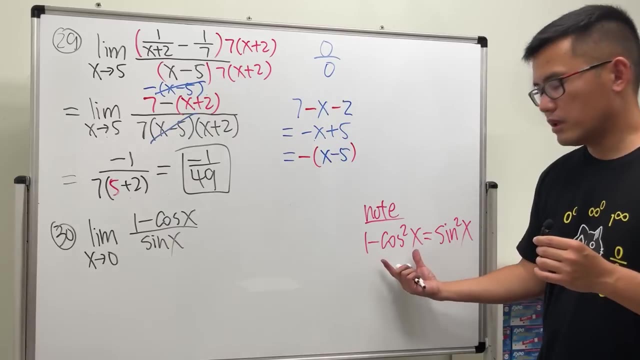 However, we do know that. Let me just put it down right here: If we have 1 minus cosine squared x, this right here is nicely equal to what Sine squared x, Yeah. So how can we go from here to here? 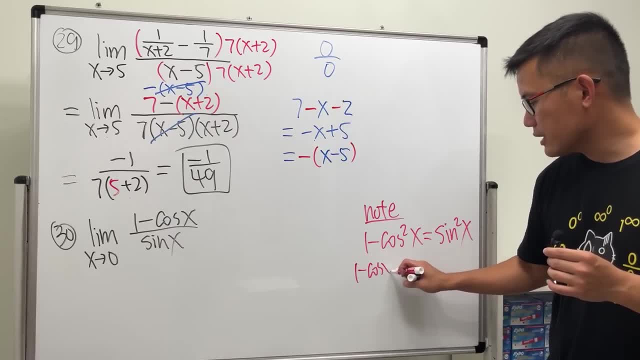 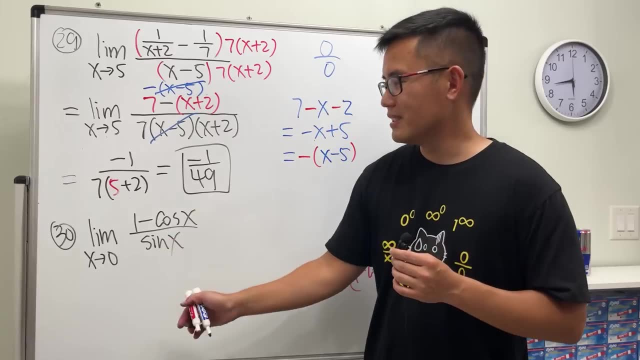 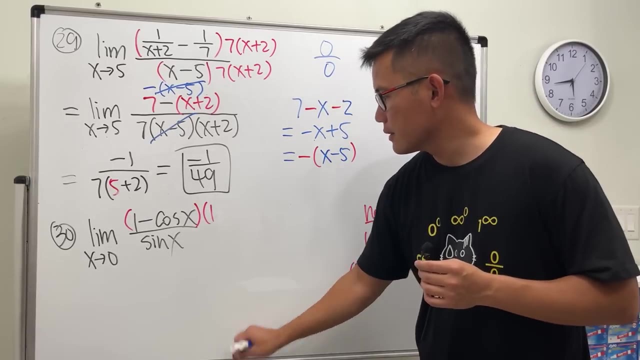 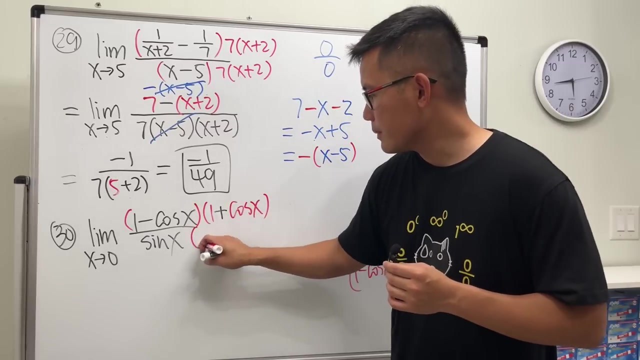 Well, this is precisely 1 minus cosine x, cosine x times 1 plus cosine x. yeah, So let's again just do the count. you get business. Take the top, multiply by 1 plus cosine x, And then, of course, we will do the same on the bottom: 1 plus cosine x. 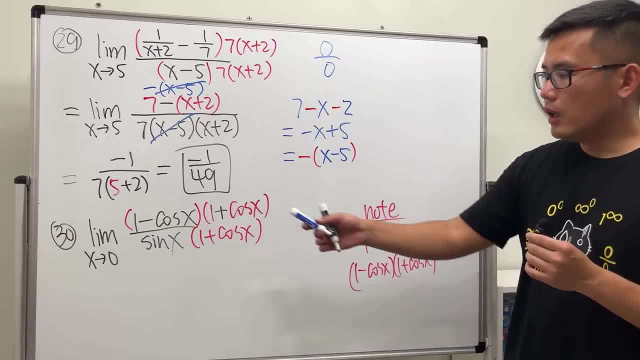 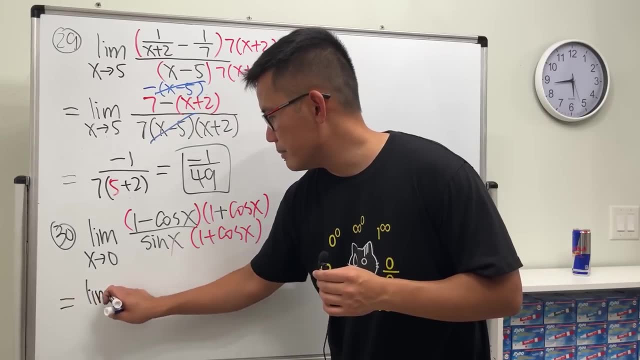 All right, And then, per our discussion here, when we do this times, that we will just get sine squared x. That's very nice. So this right here is the limit as x approaching 0.. All in all, the top is sine squared x. 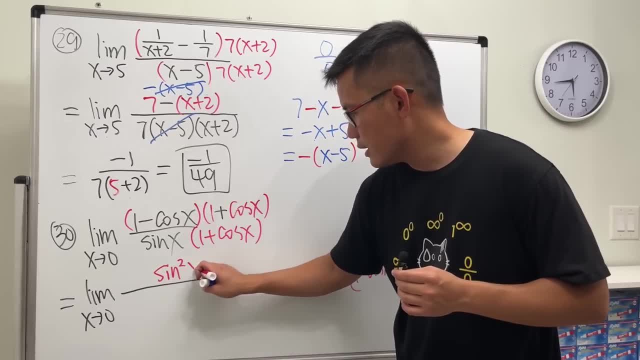 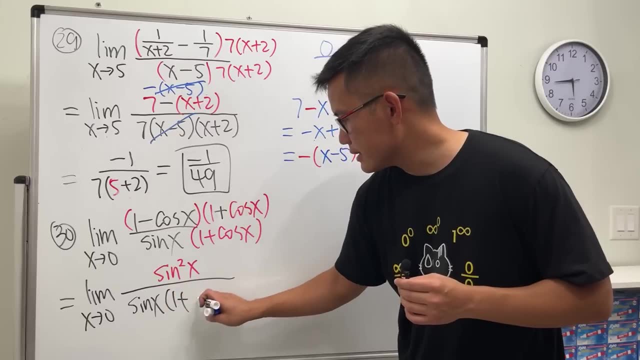 I'm just going to put that down in red. And then we have what? Here we have the sine x, And then here we have the 1 plus cosine x. Oh, by the way, I forgot to mention. 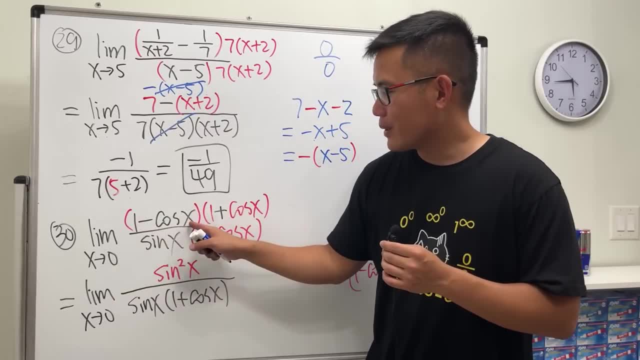 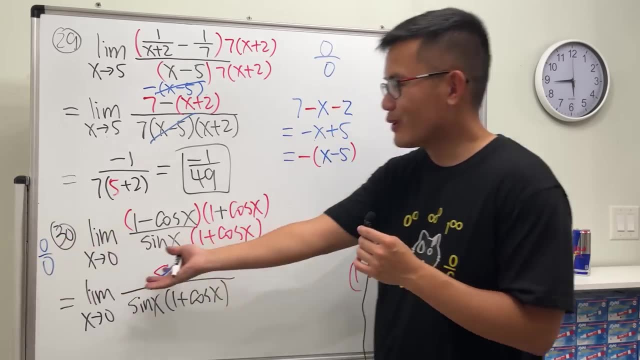 The reason that we have to do this is because when we put 0 into cosine, cosine x is 1.. 1 minus 1 is 0. When we put 0 in here, sine of 0 is 0. So yeah, it was a 0 plus 0 situation. 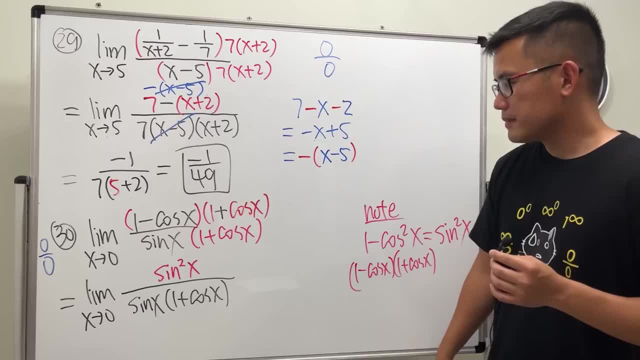 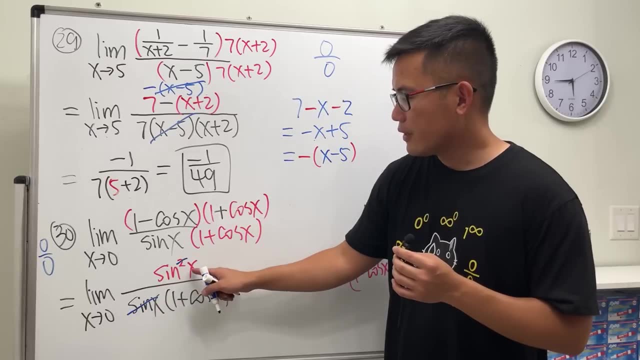 That's why we bothered to do this. Have a good habit, guys. Anyway, once we get to here, what we can do is just cancel the sine and then cancel that, So we have sine of x on the top over that on the bottom. 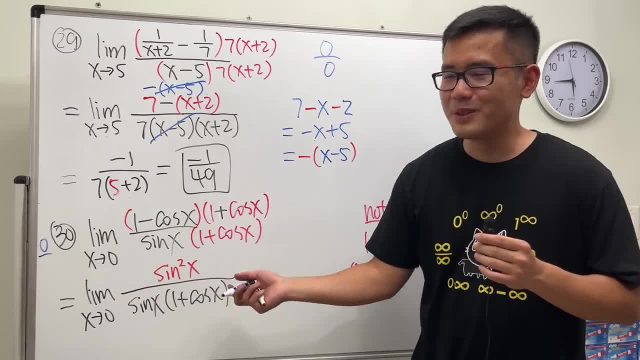 1 is 0. When we put 0 in here, sine of 0 is 0. So, yeah, it was a 0 plus 0 situation. That's why I bothered to do this. Have a good habit, guys. 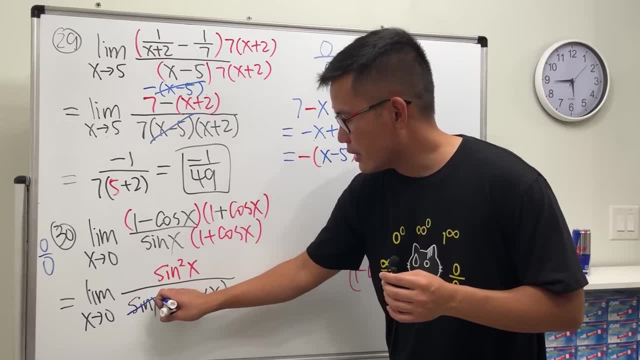 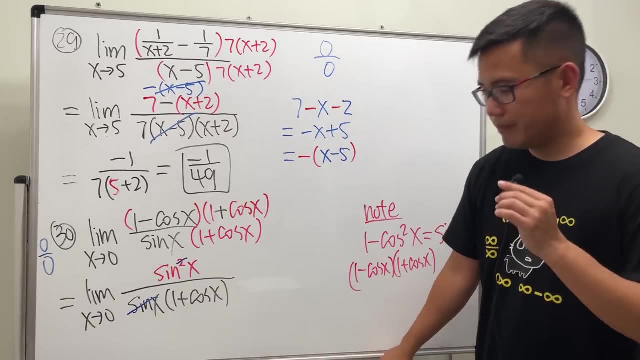 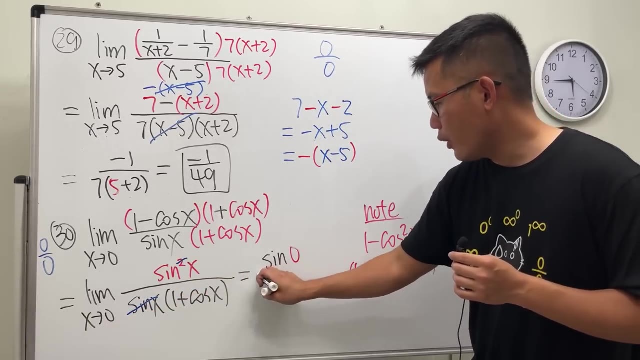 Anyway, once we get to here, what we can do is just cancel the sine and then cancel that, So we have sine of x on the top over that on the bottom. Then We can go ahead and put 0 in here. So we are looking at sine of 0 over 1 plus cosine of 0. 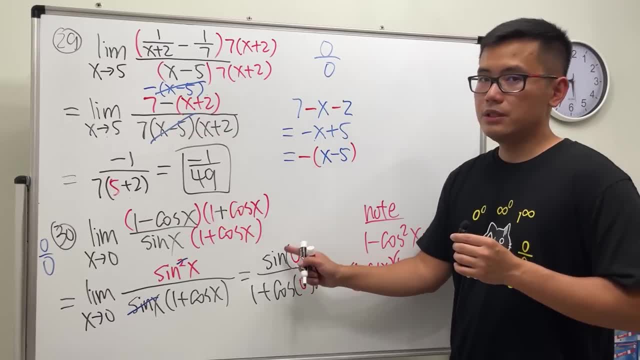 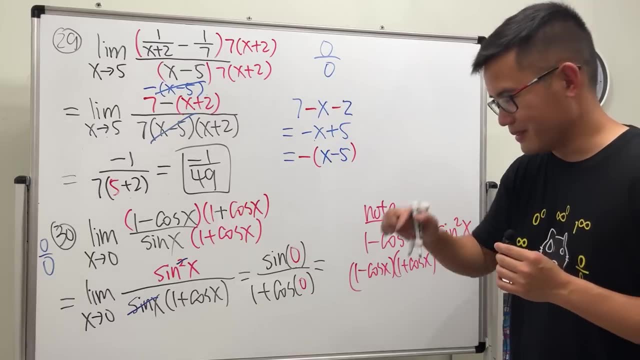 But you know what? Sine of 0 is 0.. Cosine of 0 is 1.. On the bottom it's just 1 plus 1, which is 2.. 0 over 2 is just 0.. 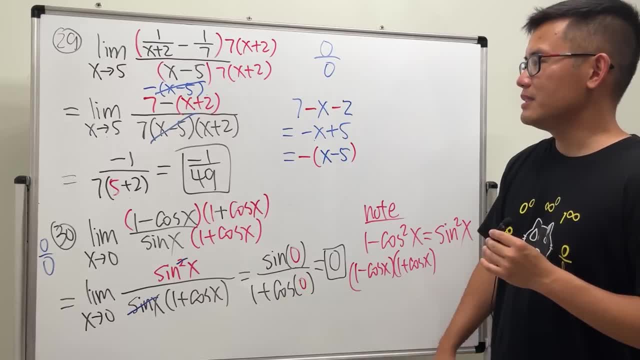 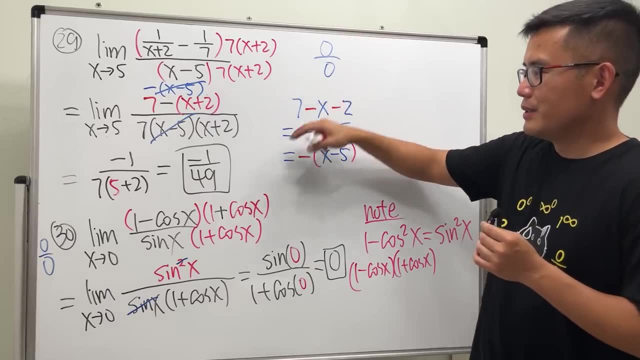 So the answer for this is 0. And hopefully by now you can see that when we have 0 for 0. The answer is 0. It's not imaginable. Like you don't know what the answer is yet, You can get a negative number, not an imaginary number. so, by the way, I shouldn't use that. 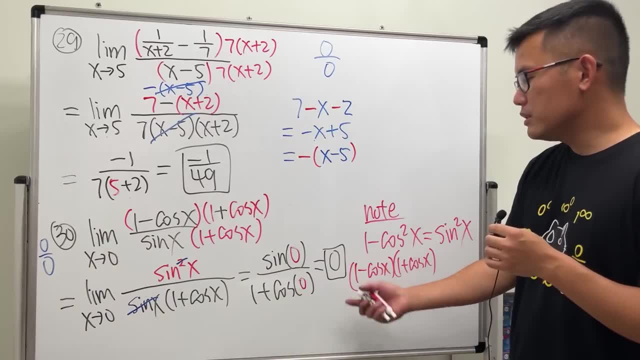 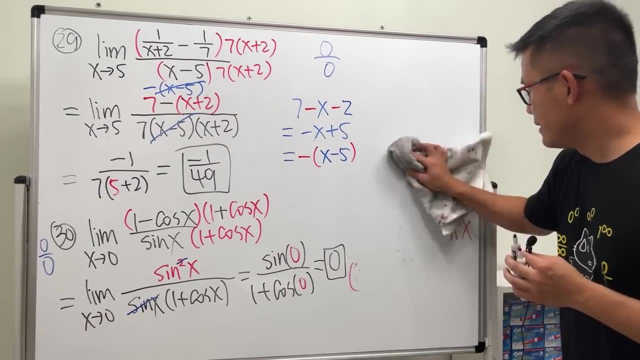 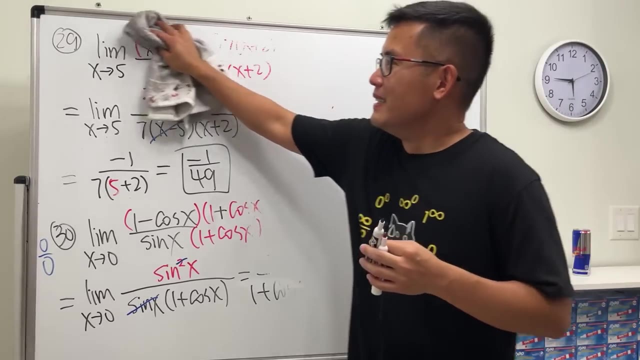 word, And then, when we have 0 over 0, it's possible to end up with 0. So many possibilities. Yeah, OK, I'm going to take the Red Bull phone in my fridge, because that Red Bull is not cold. 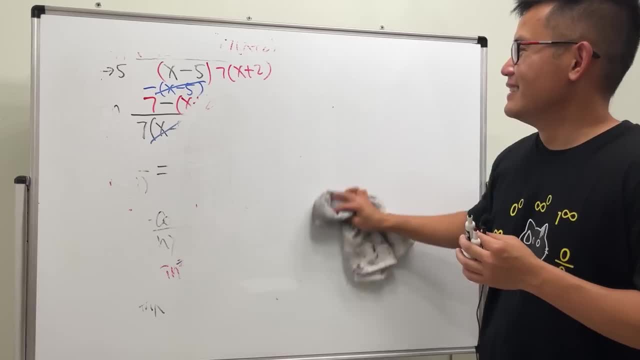 anymore, So I don't know why I took it out. Yeah, Anyway. Yeah, it's the summer, That's why, Especially when you have no AC. Anyway, I'm going to put this down here And I'll also check. 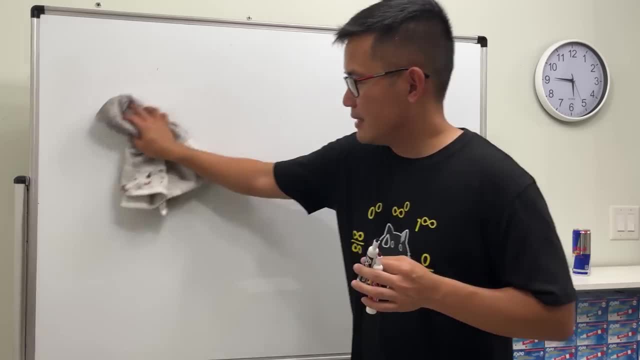 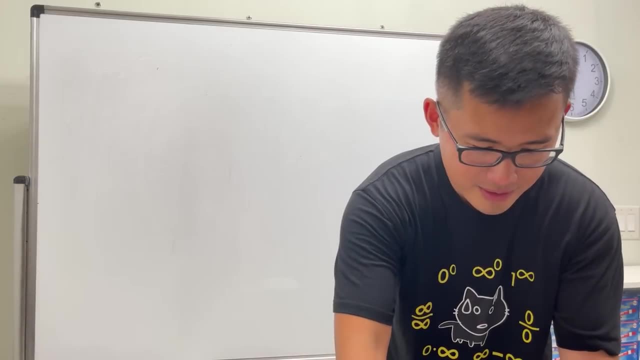 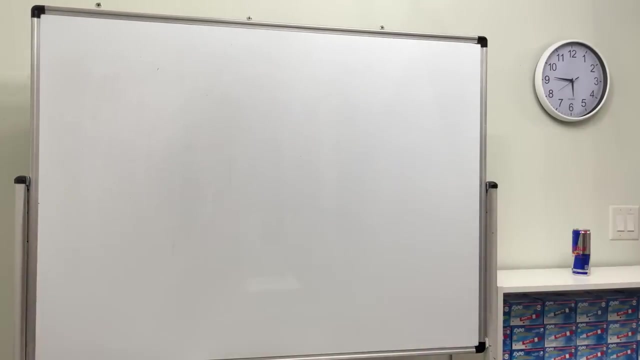 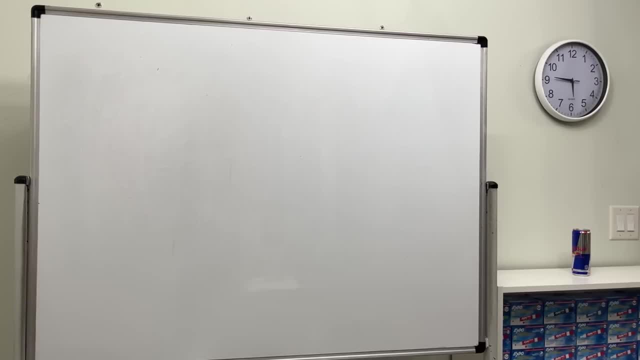 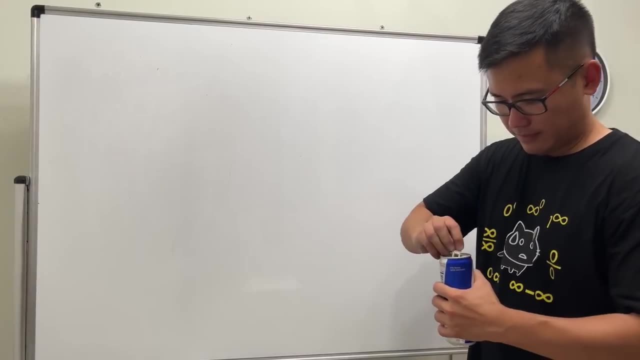 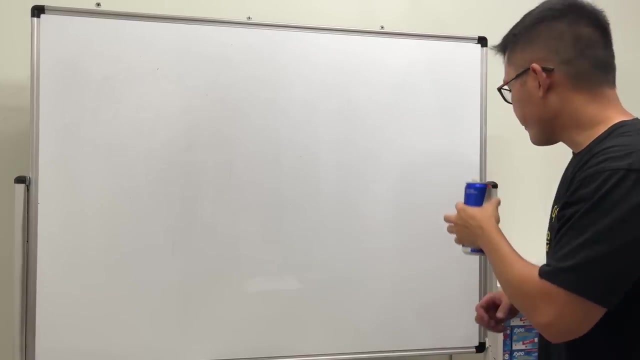 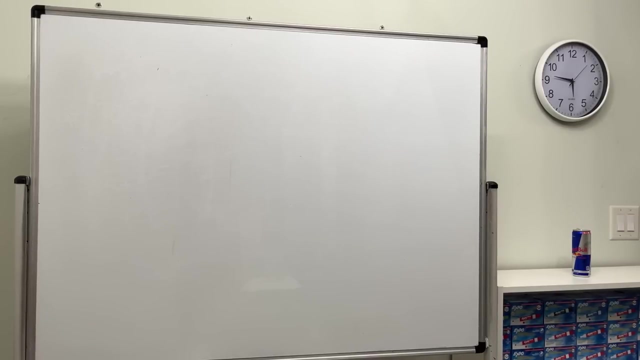 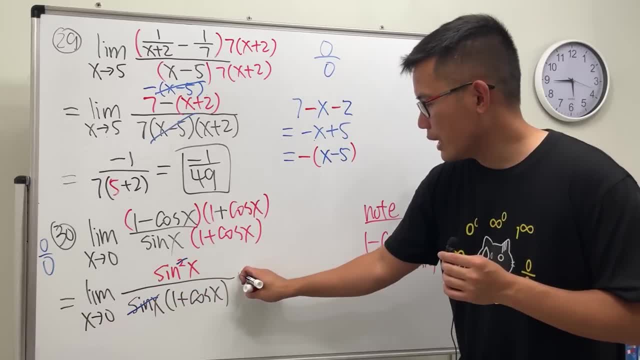 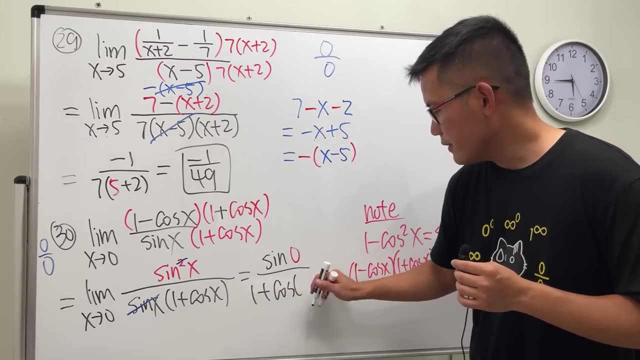 Then we can go ahead and put 0 in here. So we are looking at sine of 0 over 1 plus cosine of 0. But you know what? Sine of 0 is 0.. Cosine of 0 is 1.. 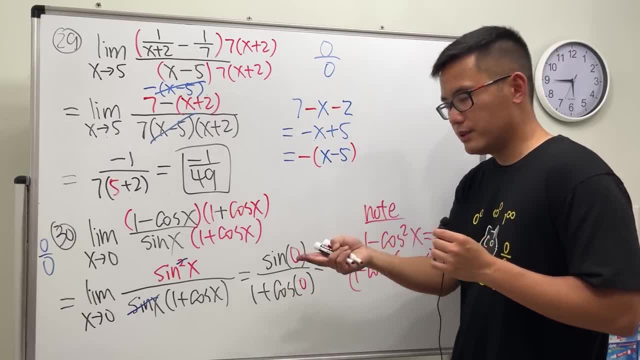 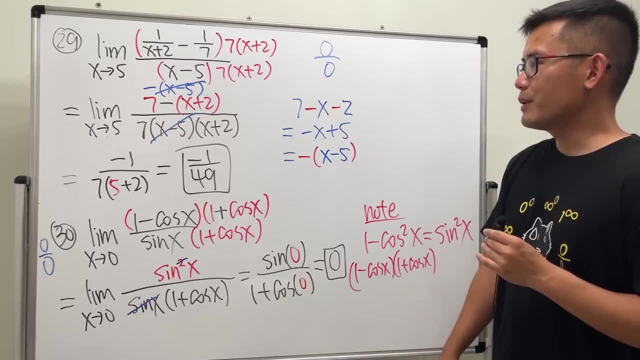 On the bottom it's just 1 plus 1, which is 2.. 0 over 2 is just 0. So the answer for this is 0. And hopefully by now you can see that when we have 0 over 0, the answer is imaginable. 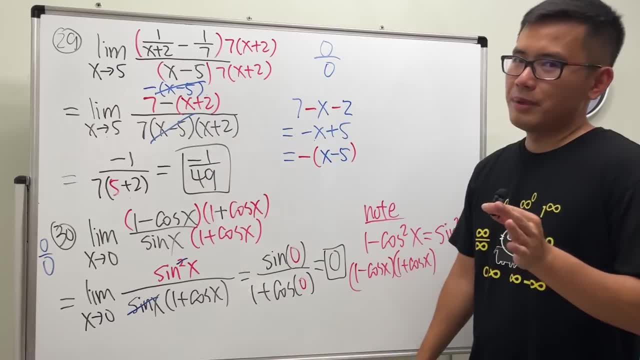 Like you don't know what the answer is yet, You can get a negative number- Not an imaginary number, by the way, It's just a number. Just use that word And then, when we have 0 over 0, it's possible to end up with 0.. 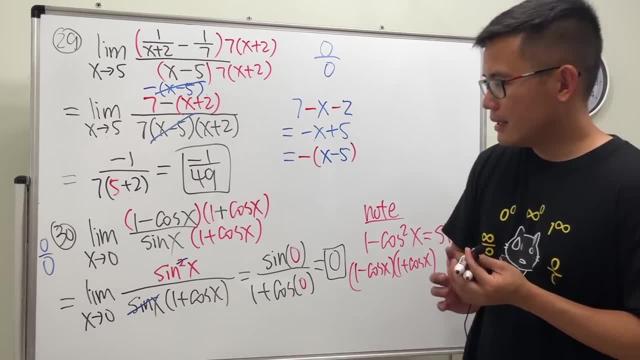 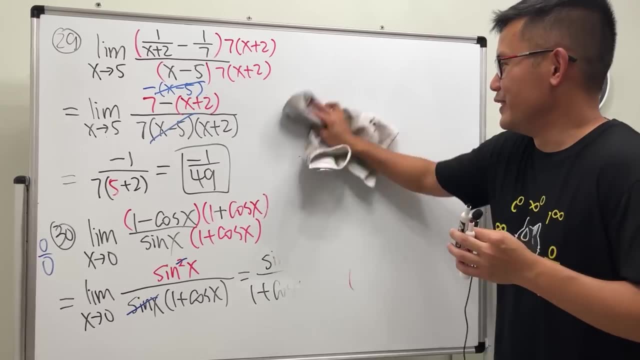 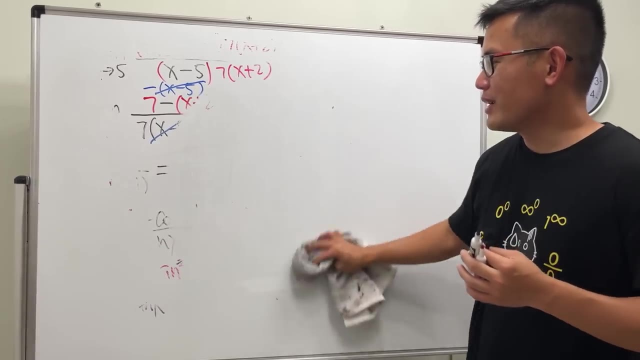 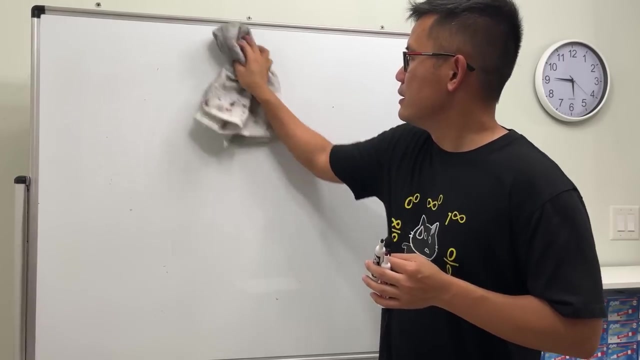 So many possibilities. Yeah, Okay, I'm going to take the Red Bull phone in my fridge, Cos that Red Bull is not cold anymore, So I don't know why I took it out. Yeah, Anyway, Yeah, it's the summer. 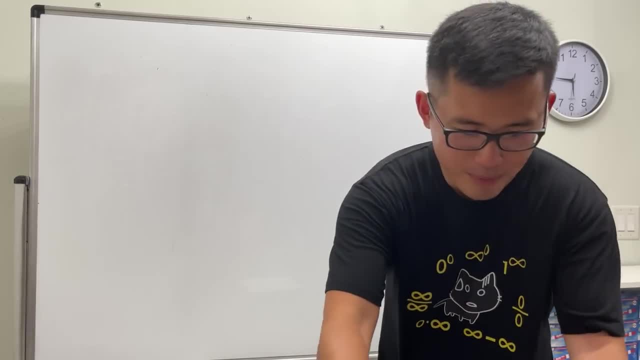 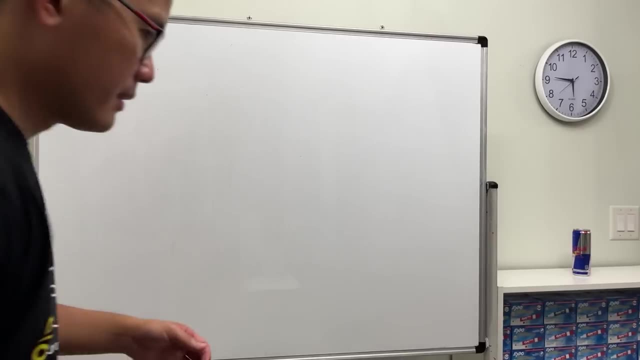 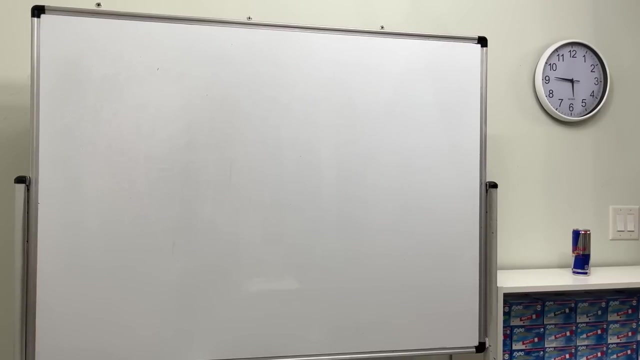 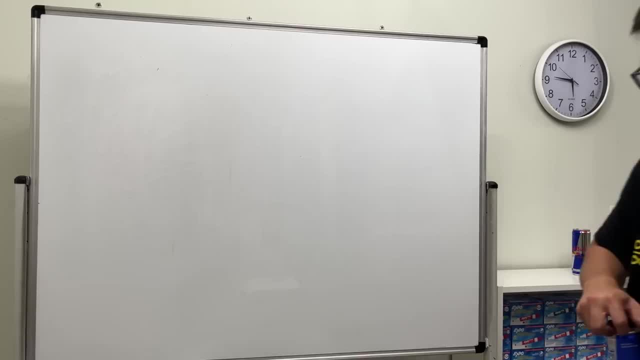 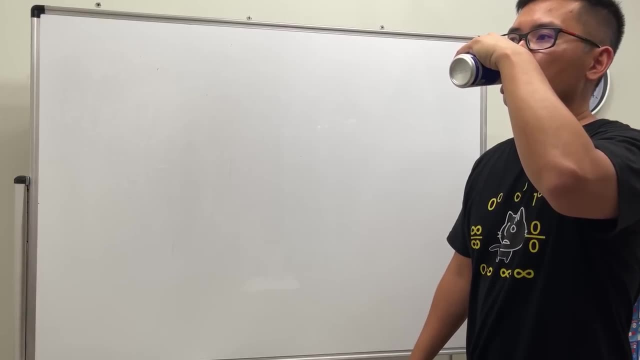 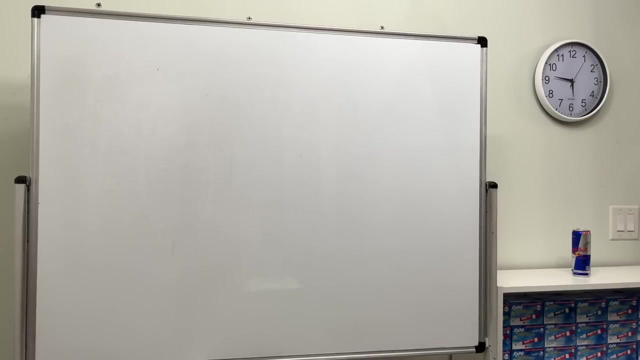 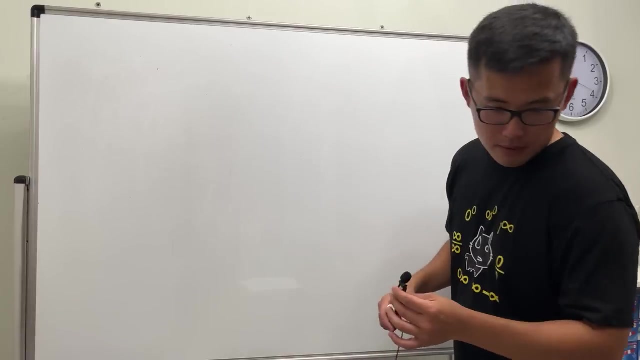 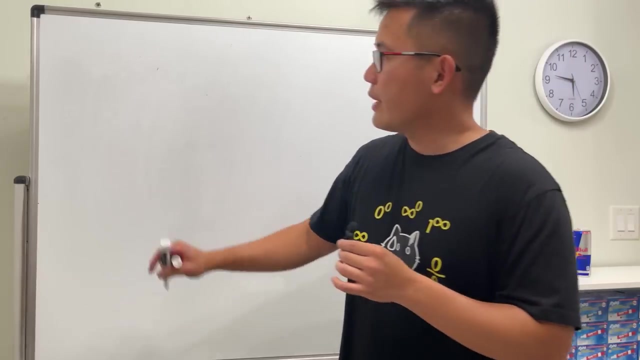 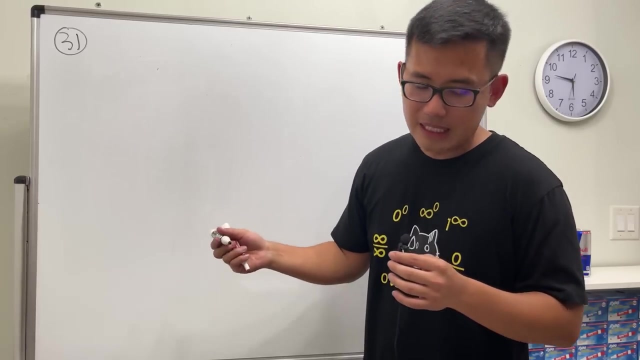 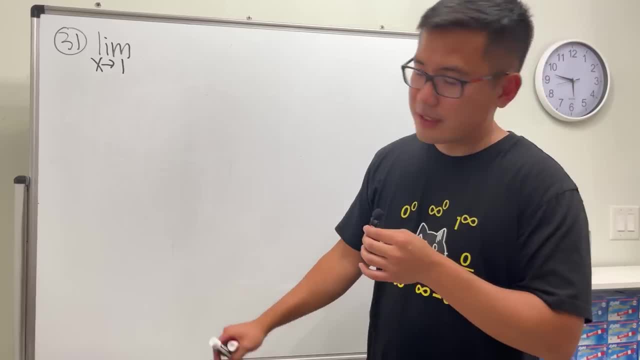 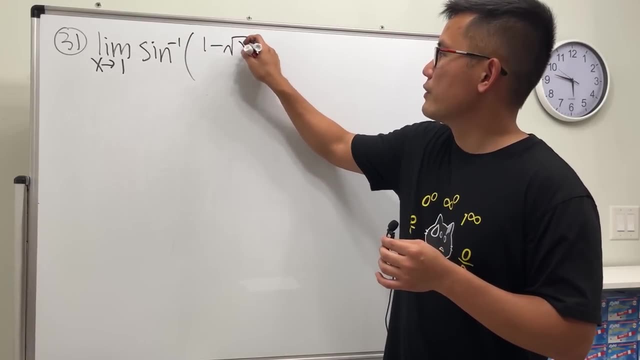 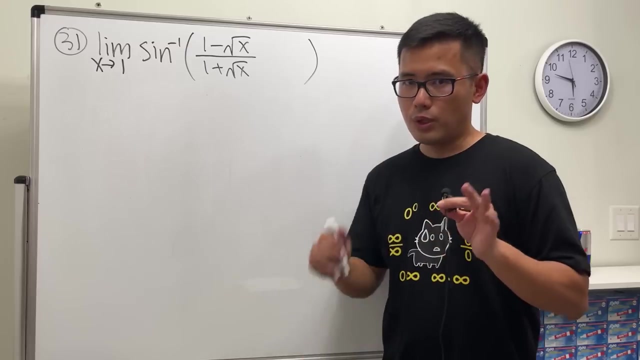 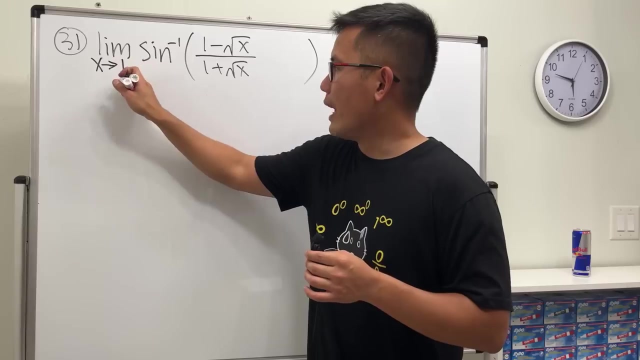 the inverse sign of the inside is one minus square root of x over one plus square root of x. yeah, you'll see why i left a big gap like that. okay, here's the deal. if we put one inside of the x here and here, oh sorry, one minus. 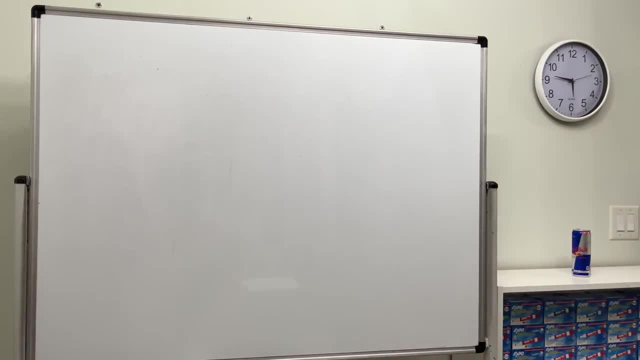 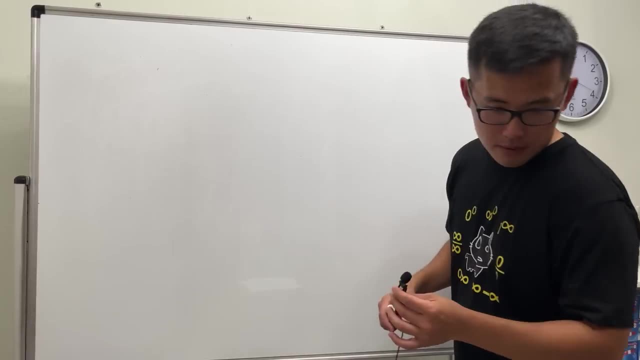 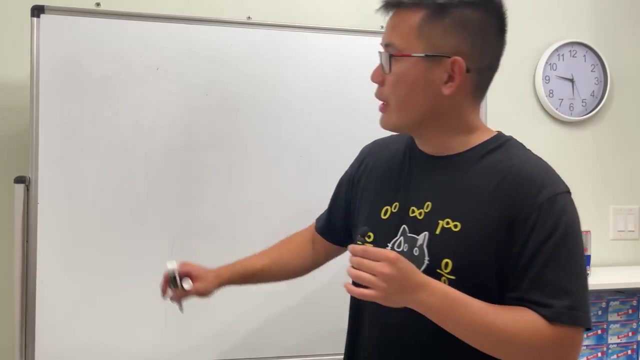 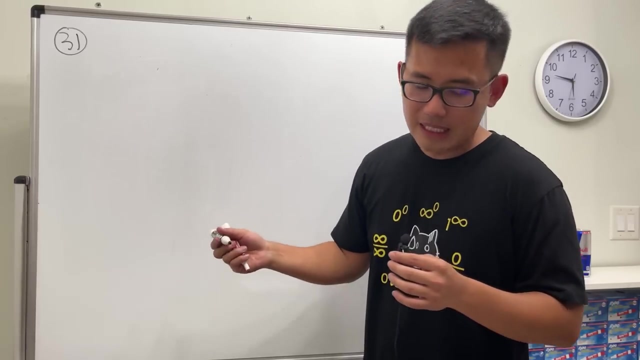 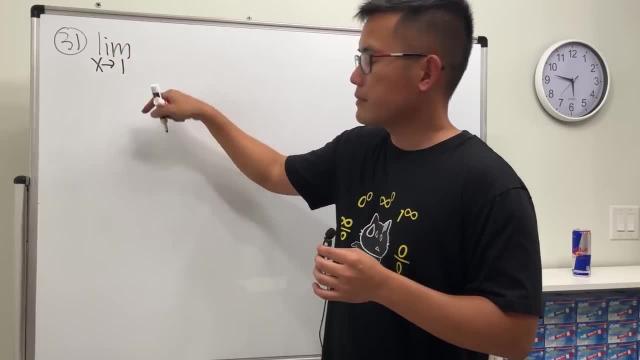 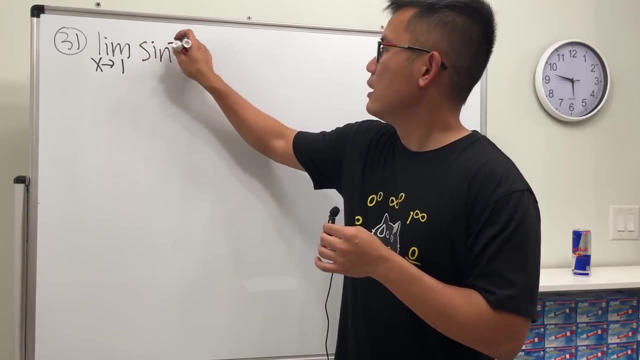 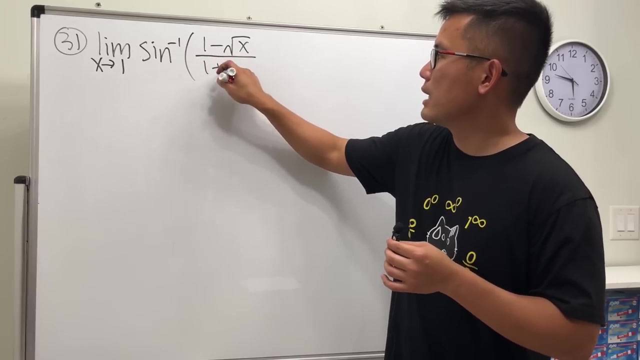 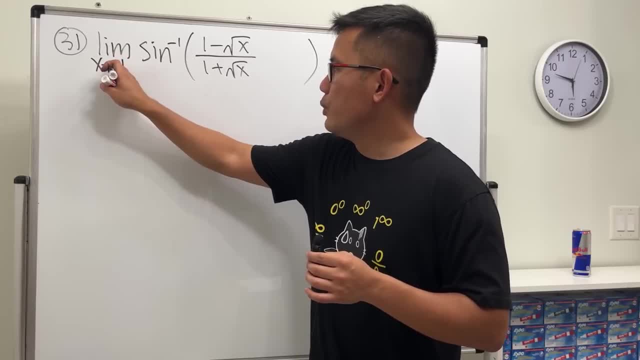 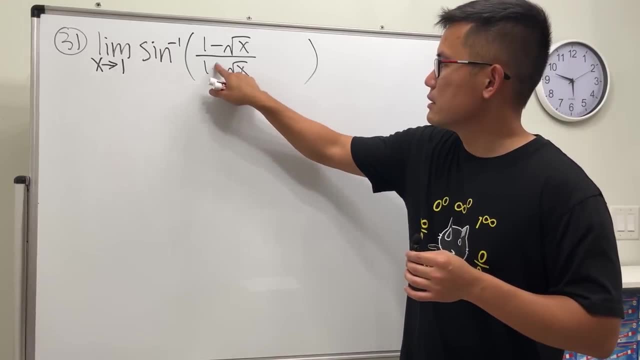 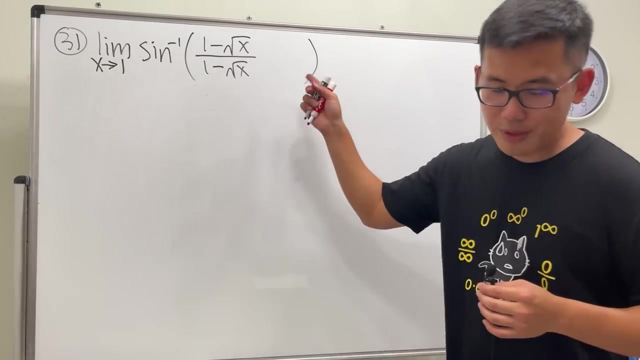 Okay, here's the deal If we put 1 inside of the x here and here, oh sorry, 1 minus x, 1 minus square root of x. I didn't mean to change the no, I wrote it down wrong. 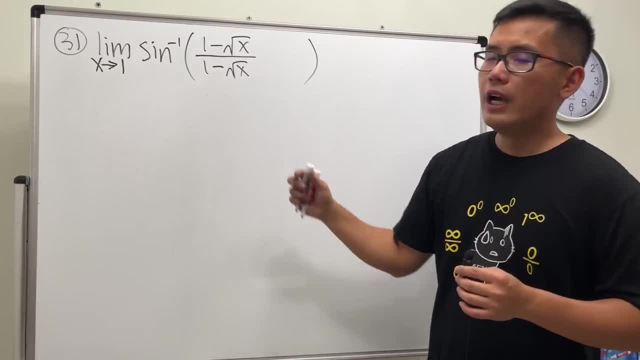 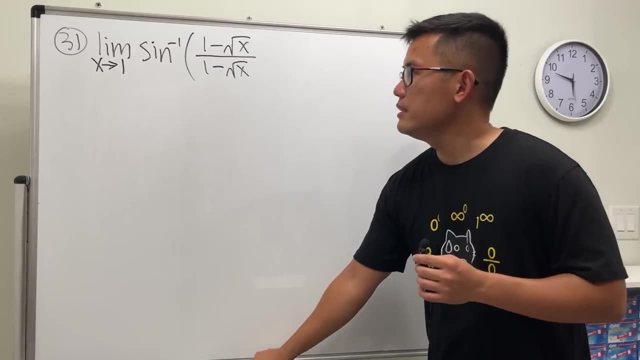 Anyway, if we put 1 into here and here, we get 0 for 0, and that's just the inside. So what we will have to do is the following: Technically, we actually do this. This is the question first. 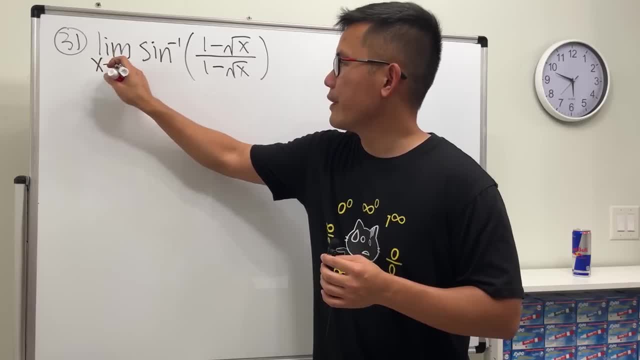 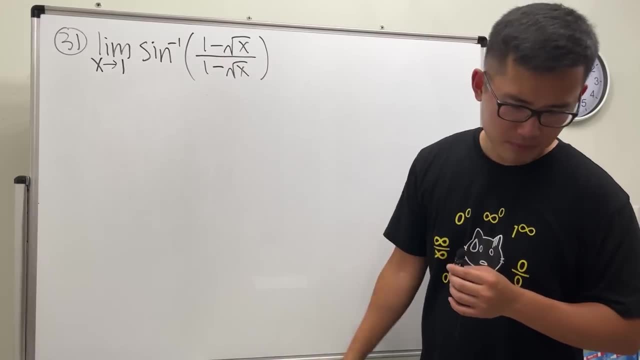 Let me just redo this. Okay, here we go. This is number 31. We have the limit as x approaching 1, inverse sine of 1 minus square root of x. No, no, no, no, no. Why am I talking about? okay? 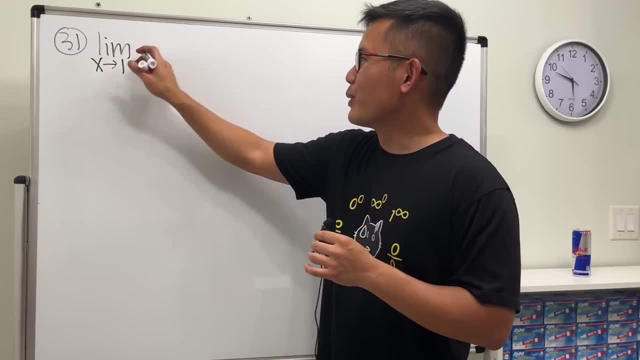 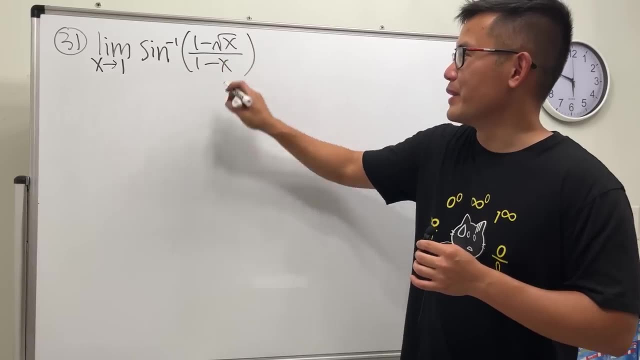 Maybe I shouldn't change the variable Anyway. number 31, the limit as x approaching 1, and we have the inverse sine of 1 minus square root of x over 1 minus x. There we go All right if we put 1 into all the x's. 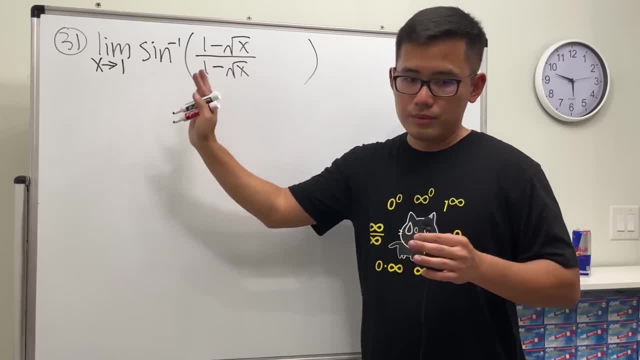 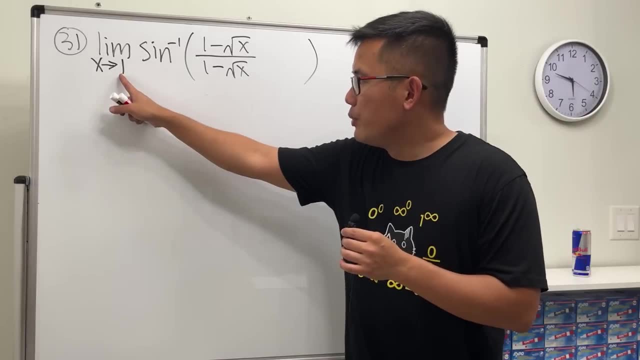 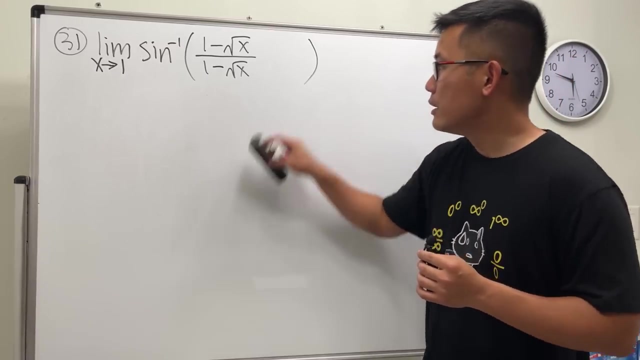 x, one, one minus square root of x. i didn't mean to change the no, i wrote it down wrong. anyway. if we put one to here and here, we get zero by zero, and that's just the inside. so what we will have to do is the following: right technically, we actually do this right. this is the question first. 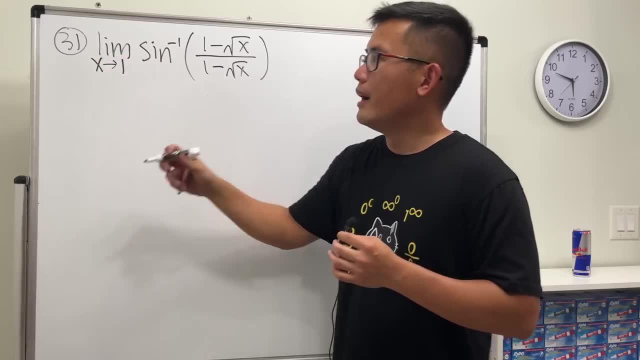 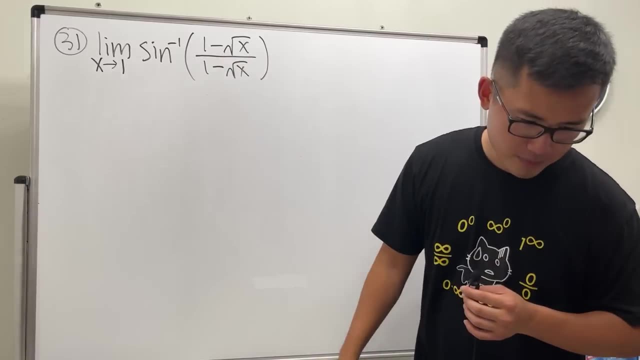 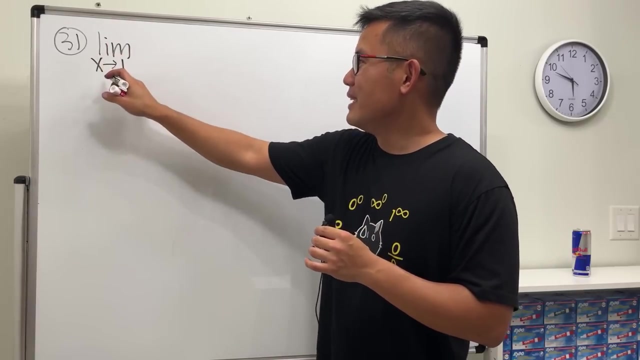 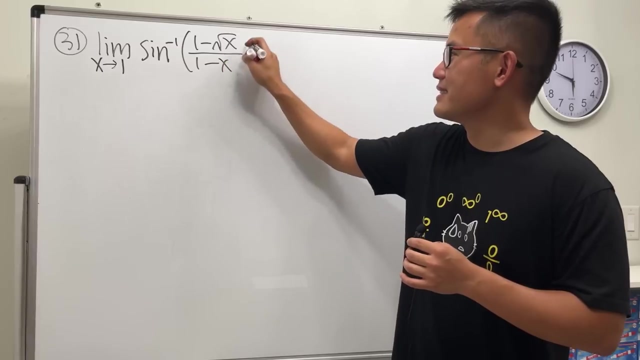 let me just redo this. all right. okay, here we go, is number 31. we have the limit as x approaching one, inverse sign of one minus square root of x. no, no, no, no, no. why am i talking about? okay, number 31, the limit as x approaching one, and we have the inverse sign of one minus square root of x over one minus x. there we go. 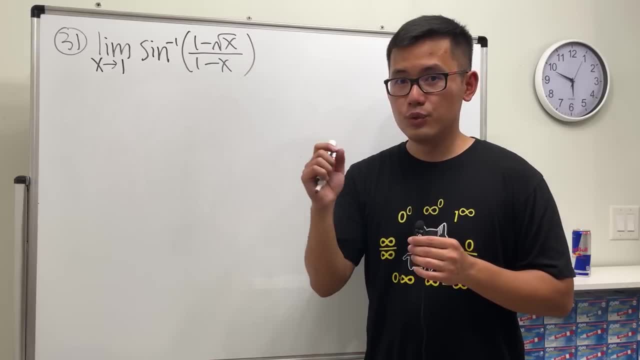 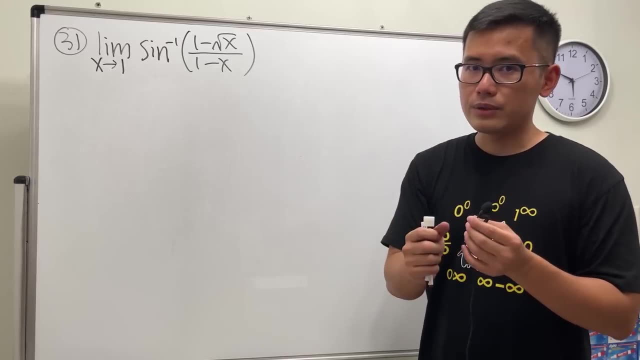 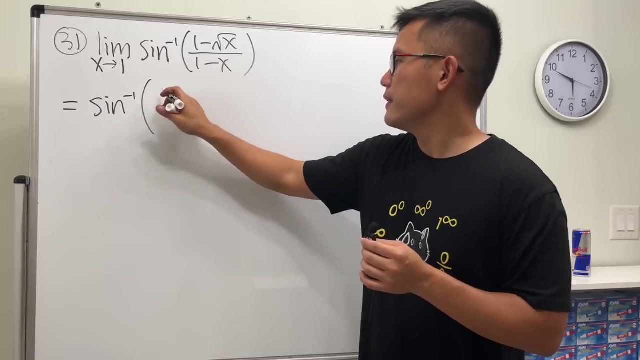 all right, if we put one into all the x's then we get zero over zero. but that's the inside. the deal is that we can actually- you look at the limit first- do the inside out. what i mean by that is the following: this is the same as saying inverse sine of the limit as x approaching 1, and then look at that. 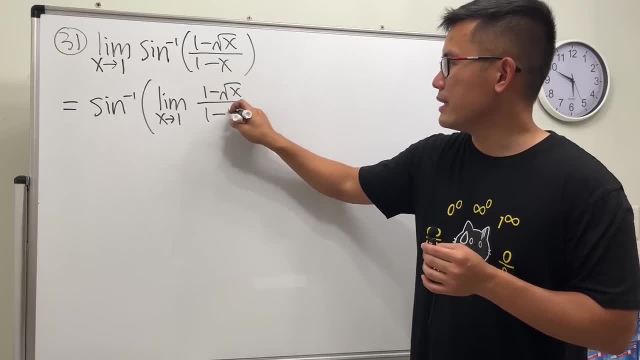 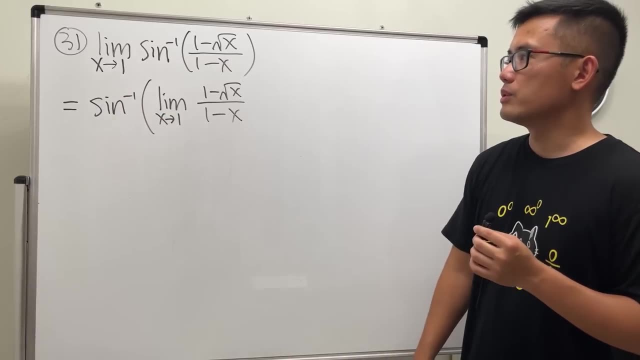 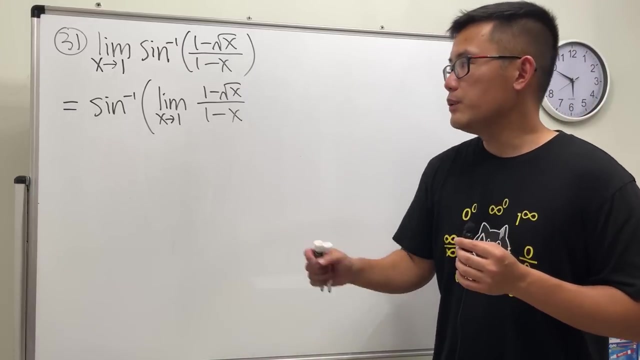 first, 1 minus square root of x over 1 minus x, and the reason i can do this is because inverse sine is a continuous function when x is approaching 1 in this particular case, so this is actually legitimate. but anyway, though, what i'm saying is that you can just do the limit inside. 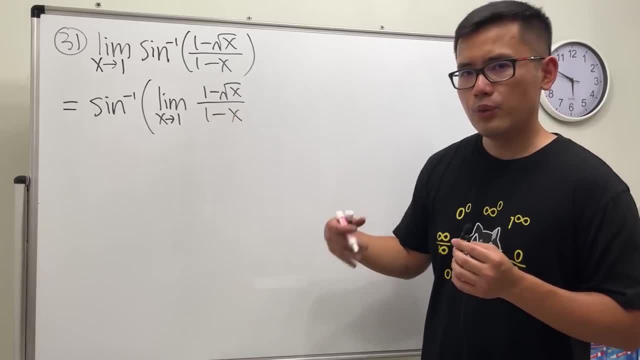 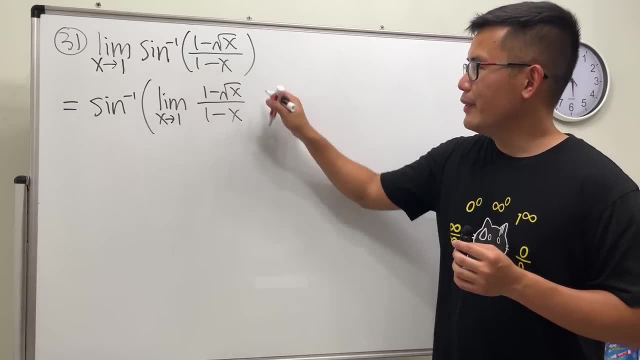 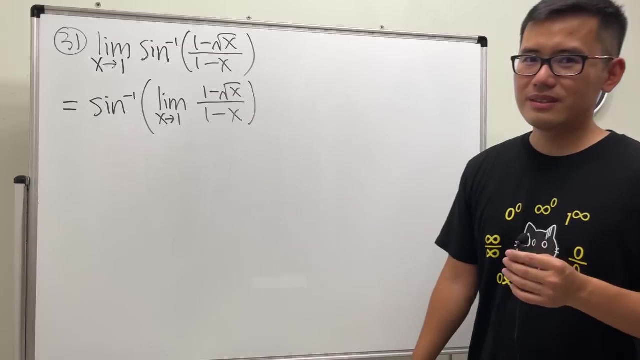 out, that's pretty much it. and for the inside- we have done this many times already- like the count, you get business, let's just go ahead. no, i'm not going to do the count you get. you can multiply one plus square root of x and also one minus square root of x. you can do that, but i want. 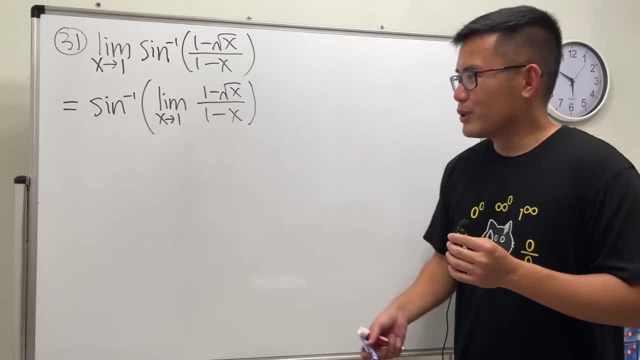 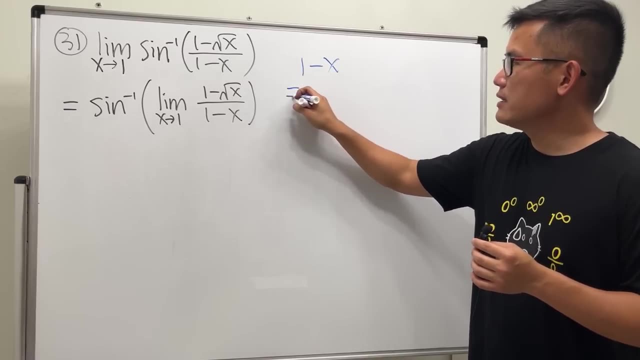 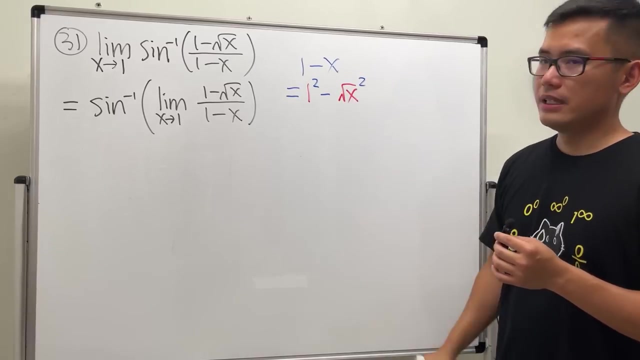 to show you something different, just so that way you have more tools that you can possibly use later on. here's the deal: when we have 1 minus x, this right here, it's the same as saying 1 square minus square root of x square. how's that? now, this is a 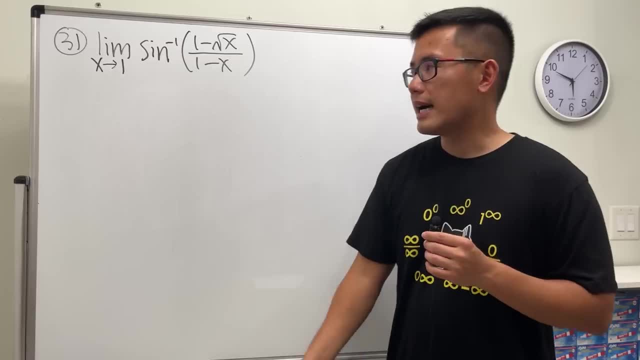 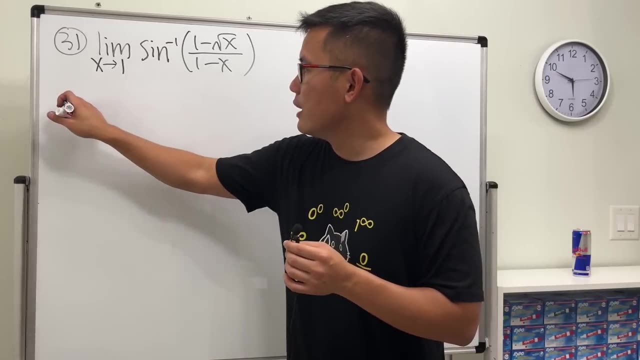 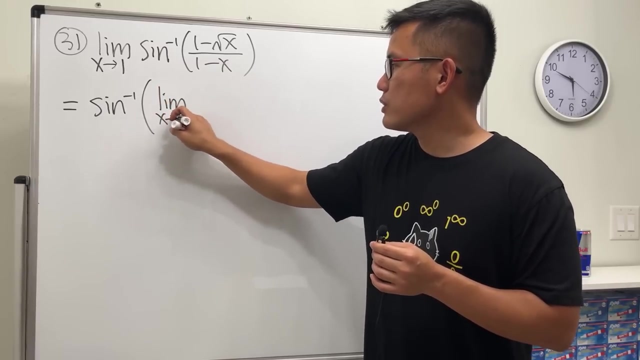 then we get 0 for 0, but that's the inside. The deal is that we can actually look at the limit first. do the inside out. What I mean by that is the following: This is the same as saying inverse sine of the limit as x approaching 1,. 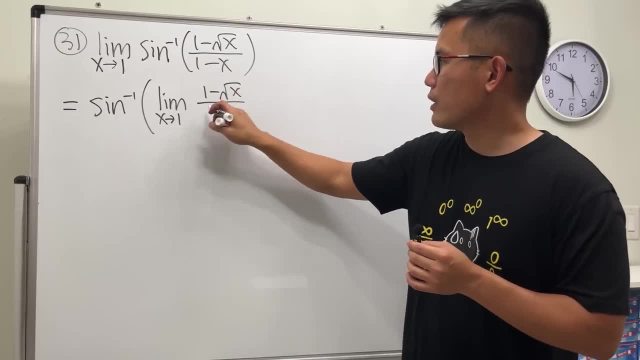 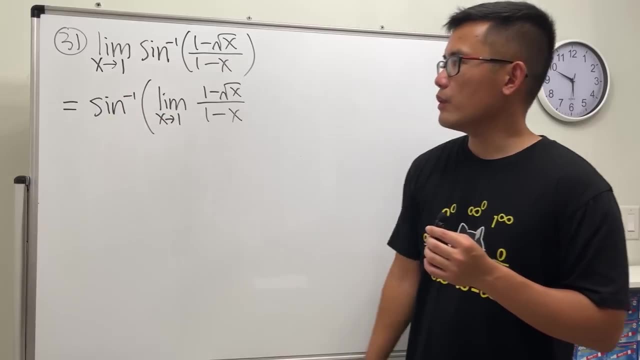 and then look at that: first, 1 minus square root of x over 1 minus x, And the reason that we can do this is because inverse sine is a continuous function when x is approaching 1 in this particular case. So this is actually legitimate. 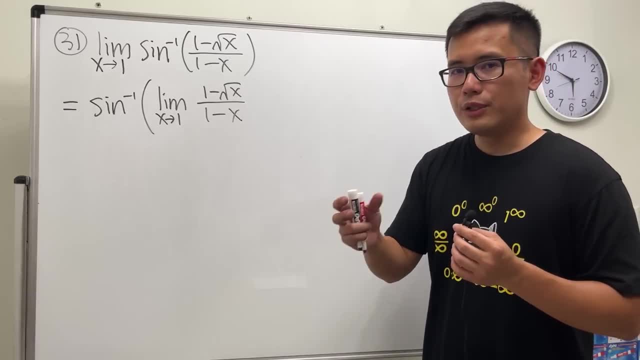 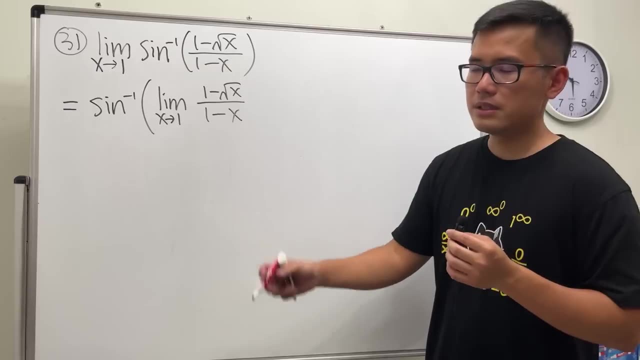 But anyway, though, what I'm saying is that you can just do a limit inside out, That's pretty much it, And for the inside- we have done this many times already, like the count-gigit business- Let's just go ahead. 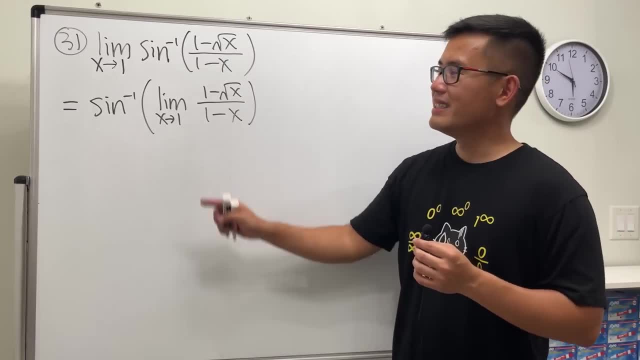 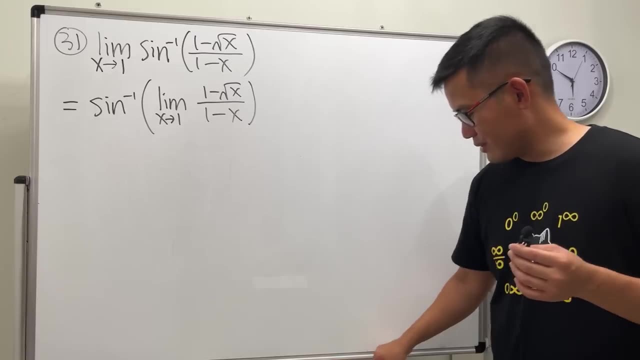 No, I'm not going to do the count-gigit. You can multiply 1 plus square root of x and also 1 minus square root of x. You can do that. But I want to show you guys something different, just so that way you have more tools. 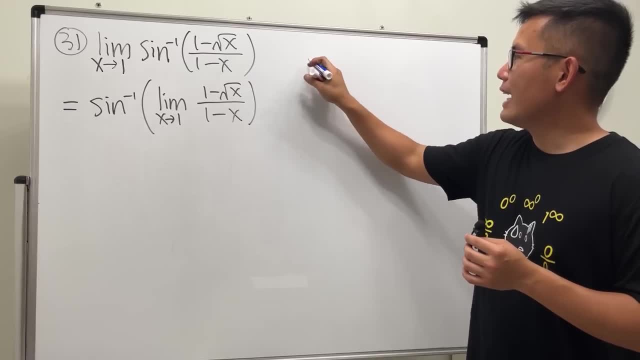 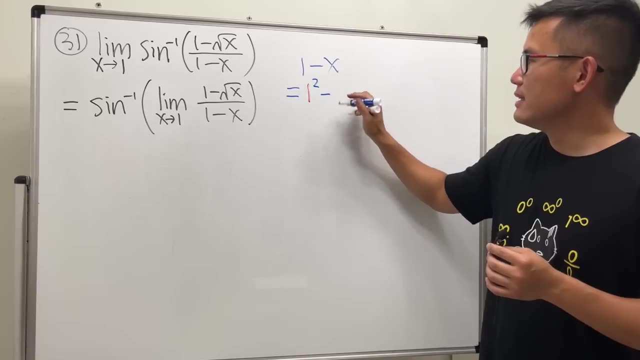 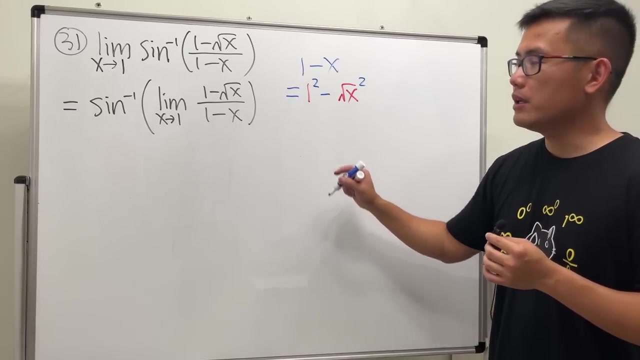 that you can possibly use later on. Here's the deal: When we have 1 minus this right here, it's the same as saying 1 square minus square root of x squared. How's that? Now, this is a difference of two squares. 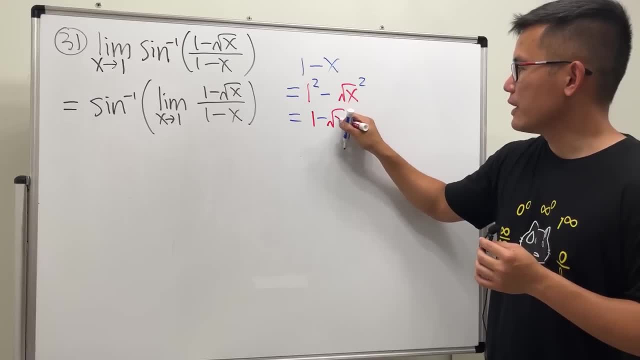 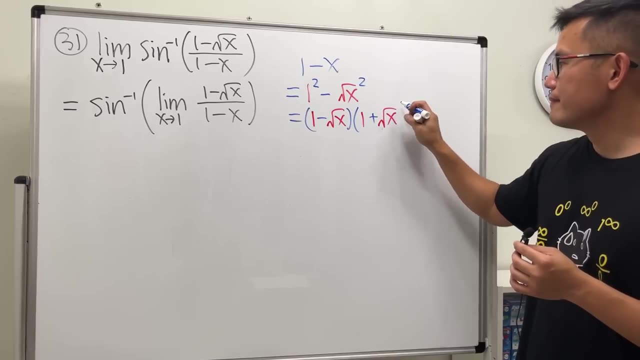 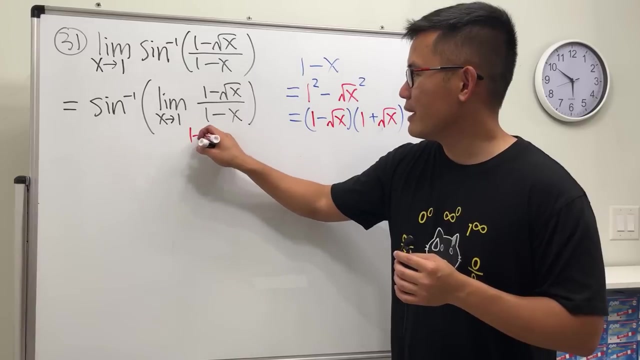 So we can say 1 minus square root of x times 1 plus square root of x. Yep, So in fact, this guy is just that, which is 1 minus square root of x And then 1 plus square root of x. 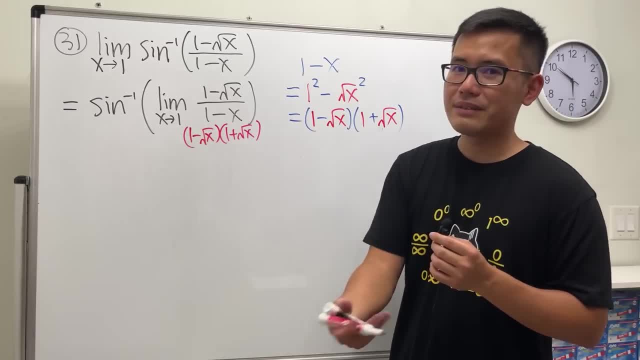 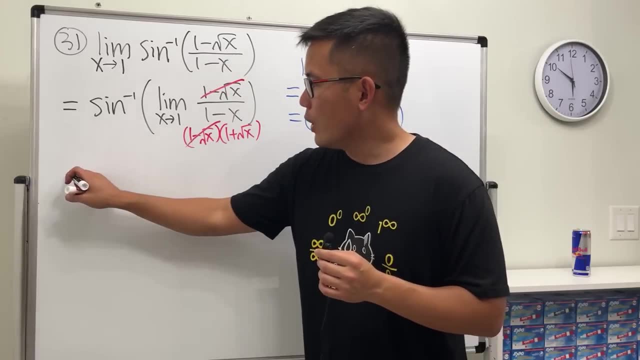 If you do the count-gigit, you will end up with the same thing like after the cancellation: Anyway, this and that cancel out very nicely. So what we are going to get is the inverse sign, And then we just have to put a 1 in here. 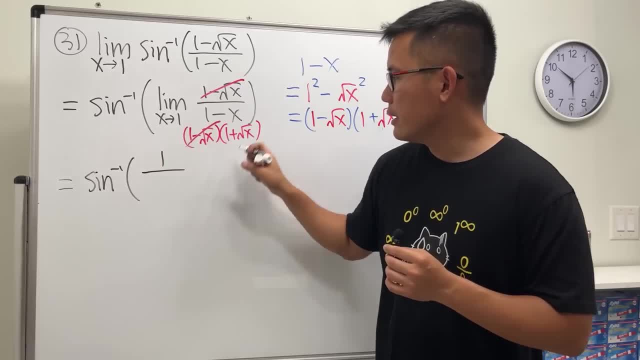 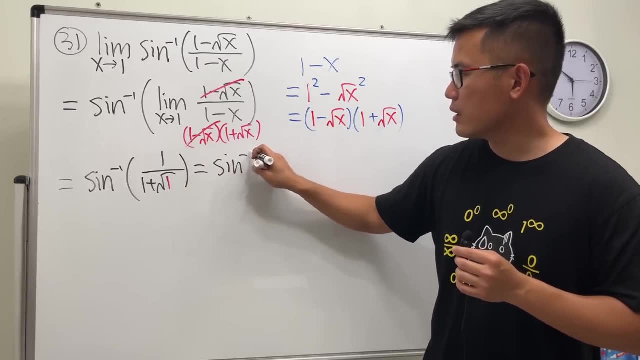 and that's on the bottom. So don't forget, we still have the 1, and then the 1 on the top, and then 1 plus Square root of 1.. And this is just inverse sign of 1 half. 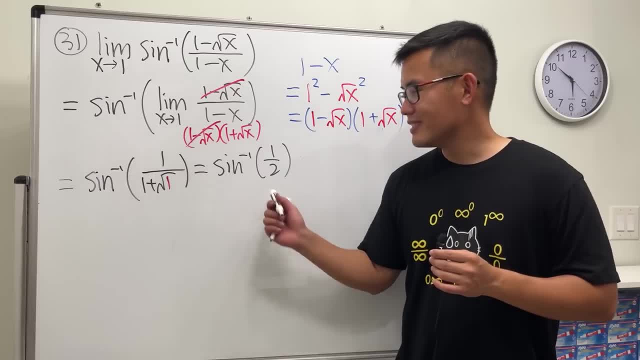 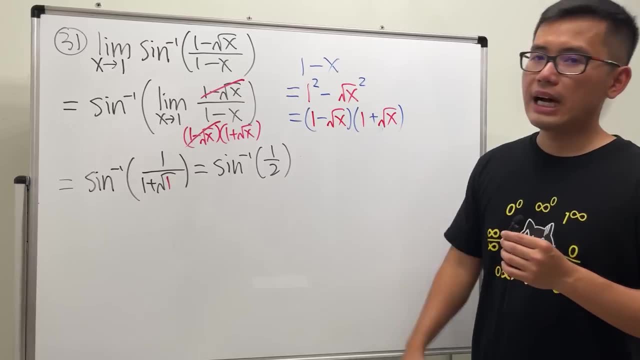 Now, I know this is the hardest part: How do we do this? The way to do it is you have to ask yourself the original sign of what angle will give us 1 half. And that's still hard. huh, I know. 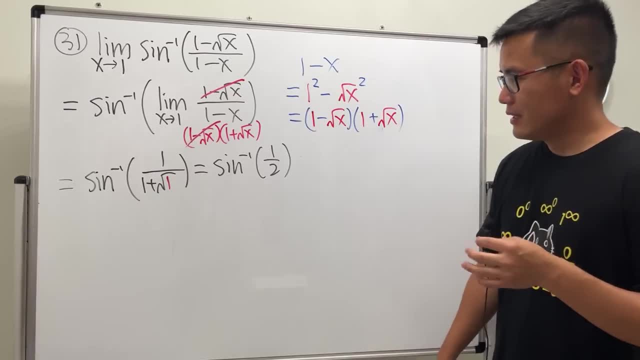 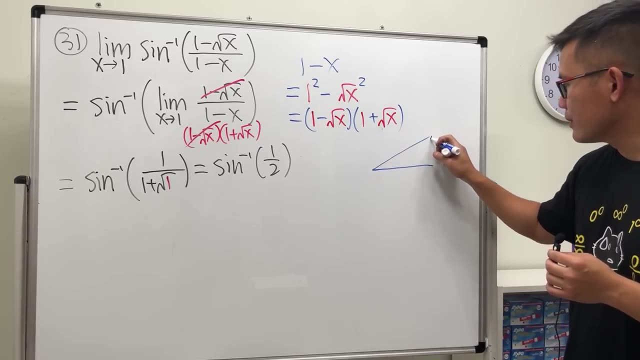 Sometimes it's hard for me too, so I will use the special triangle. So sine is the opposite over hypotenuse. So here's the deal. Here is the triangle 1 over 2.. We see we have a special right triangle. 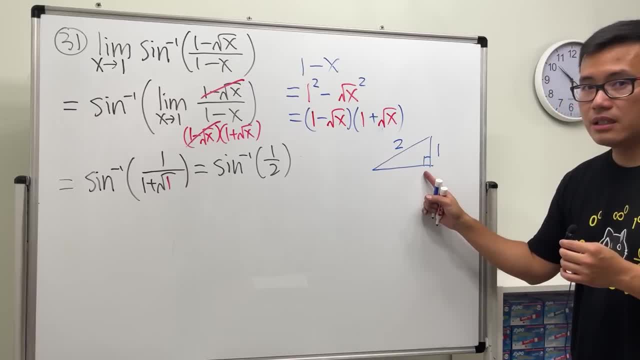 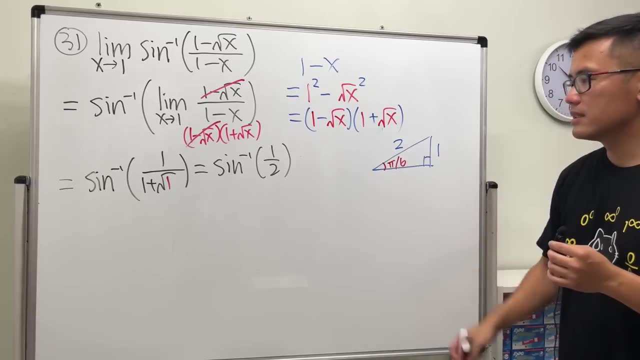 and the angles are what? 30,, 60,, 90. This is 30 degrees. This is the angle. 30 degrees is the same as pi over 6.. So, ladies and gentlemen, inverse sine of 1 over 2 is pi over 6.. 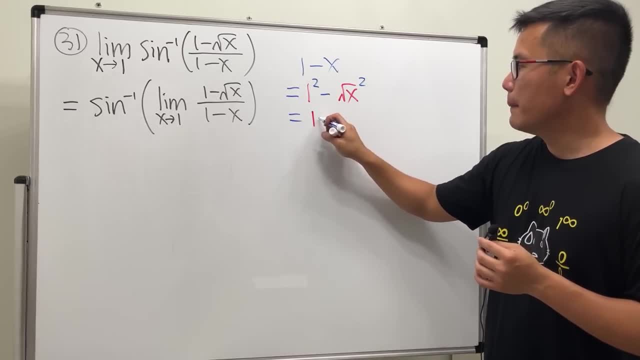 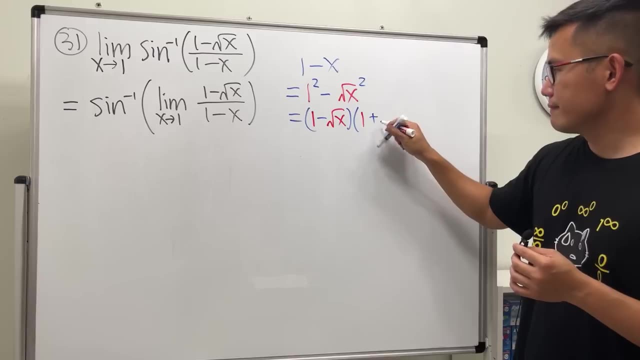 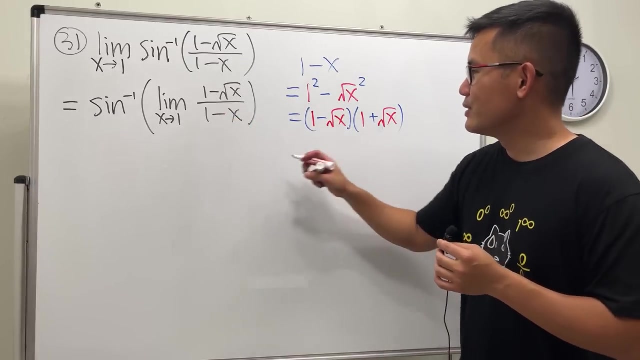 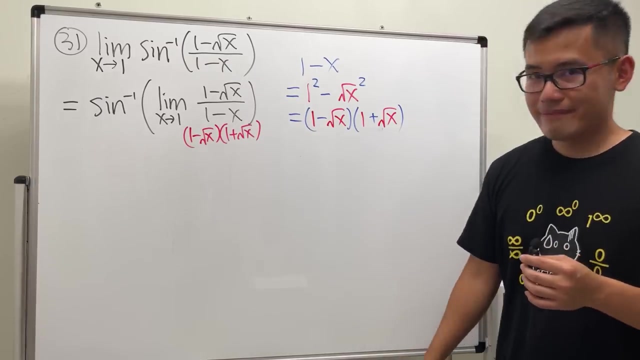 difference of two squares. so we can say 1 minus square root of x times 1 plus square root of x. yep, so in fact this guy is just that, which is 1 minus square root of x and then 1 plus square root of x. if you do the count you get. you end up with the same thing like this: after the cancellation: 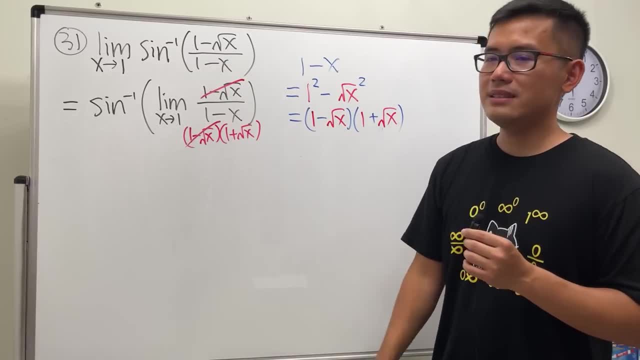 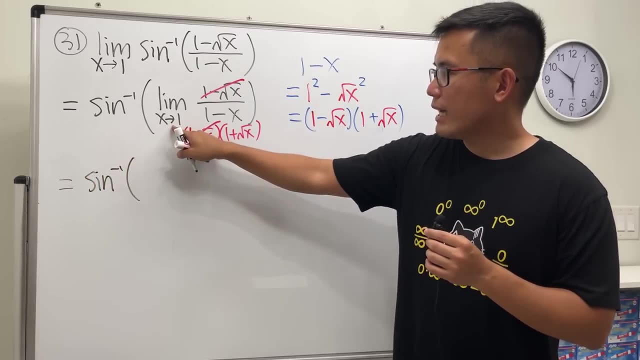 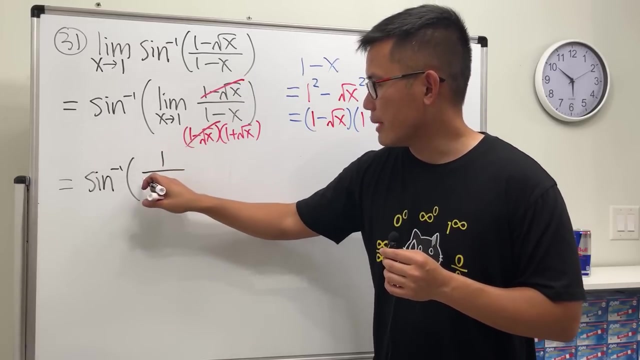 anyway, this and that cancel out very nicely. so what we are going to get is the inverse sine, and then we just have to put a 1 in here and that's on the bottom. so don't forget, we still have the 1, and then the 1 on the top, and then 1 plus square root of 1. 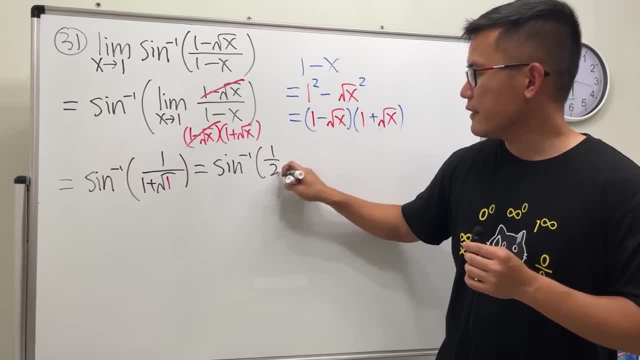 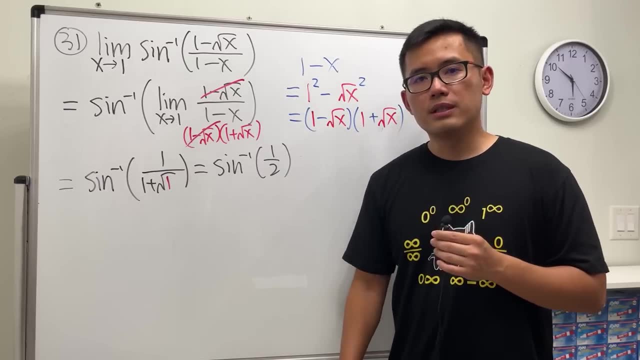 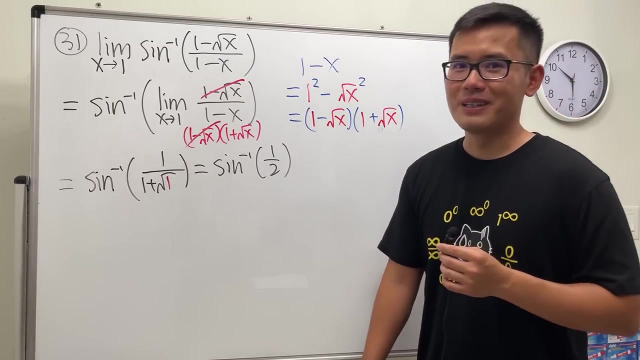 and this is just inverse sine of 1 half. now i know this is the hardest part: how do we do this? the way to do it is you have to ask yourself the original sign of what angle will give us one half. and that's still hard, huh? i know. sometimes it's hard for me too, so i will use the 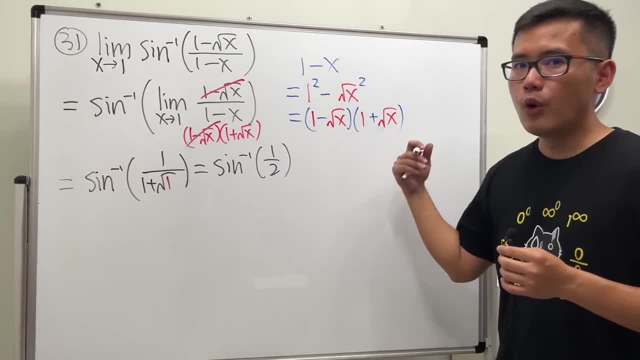 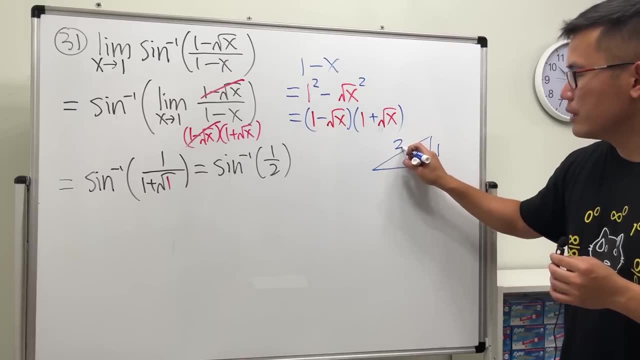 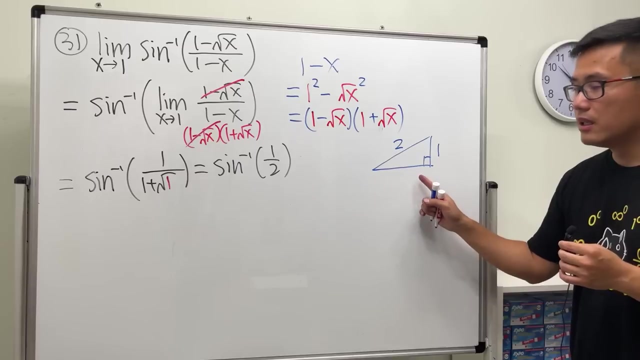 special triangle. sine is the opposite over hypotenuse. so here's the oh, here is the triangle, one over two. we see we have a special right triangle and the angles are what? 30, 60, 90.. this is 30°. this is the angle. 30° is the same as pi over 6.. 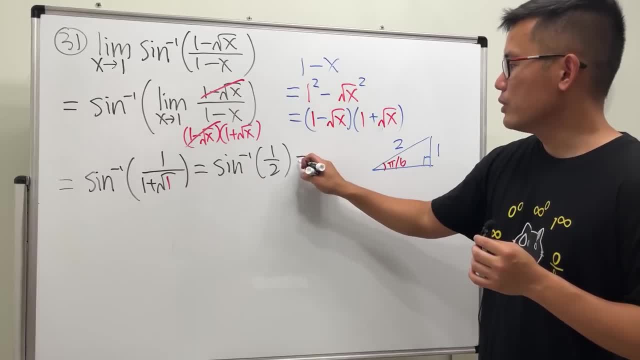 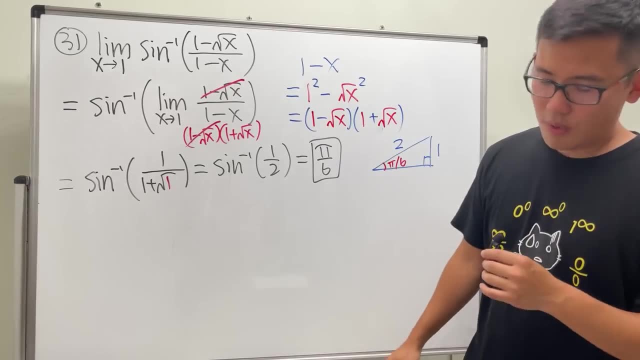 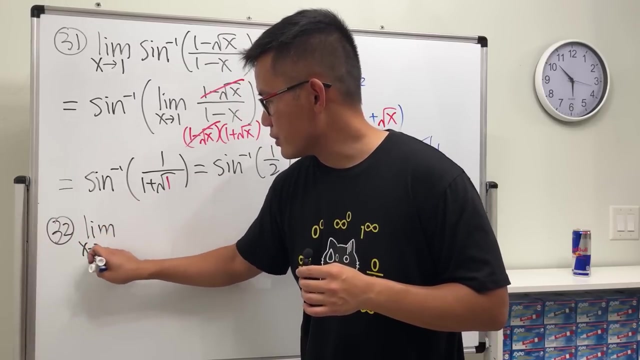 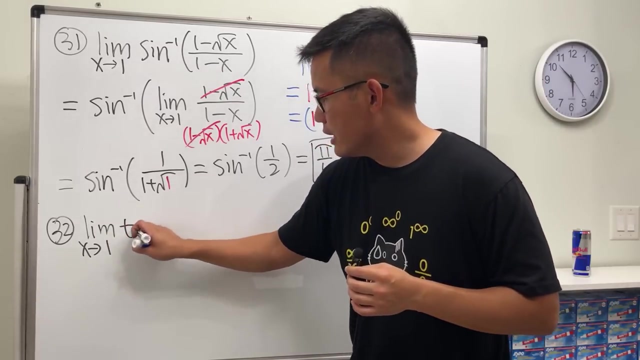 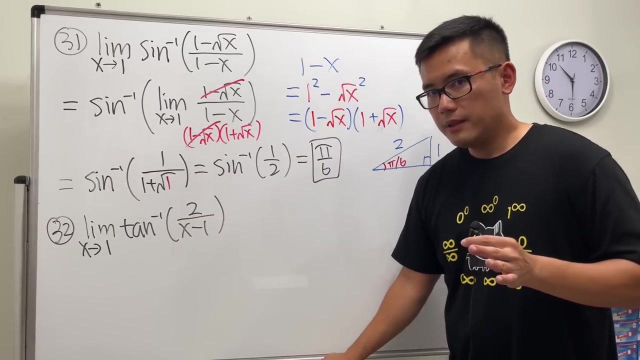 so, ladies and gentlemen, inverse sine of 1 over 2 is pi over 2.. over 6, next one number, 32. all right, here we have the limit as X approaching 1, and then here I am going to give you guys inverse tangent of 2 over X minus 1. okay, 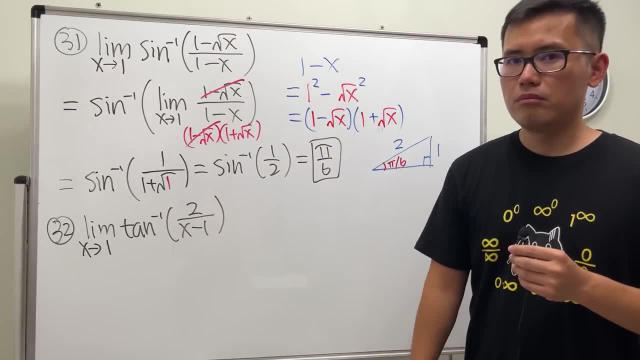 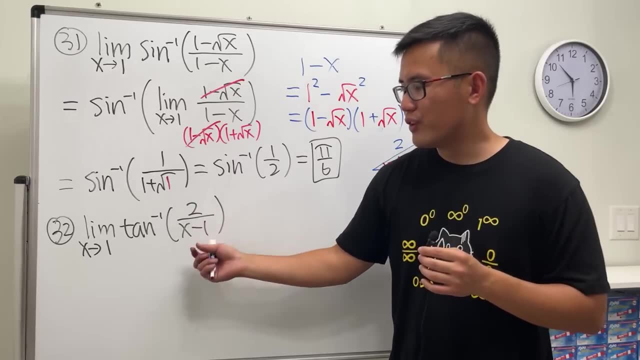 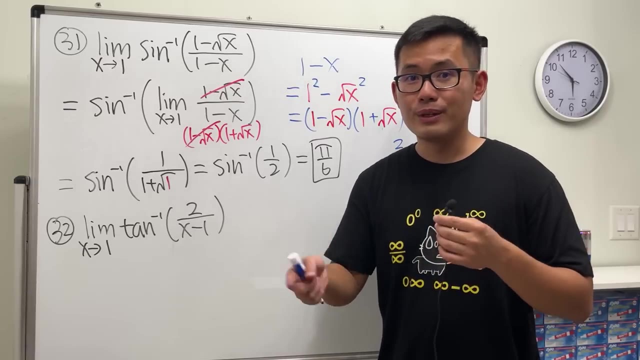 can we do the same that we did earlier? not really in the following sense, because you see, if we put 1 inside here we get 2 over 0. is it positive infinity or is it negative infinity? we will have to do what. yeah, we will have to consider. 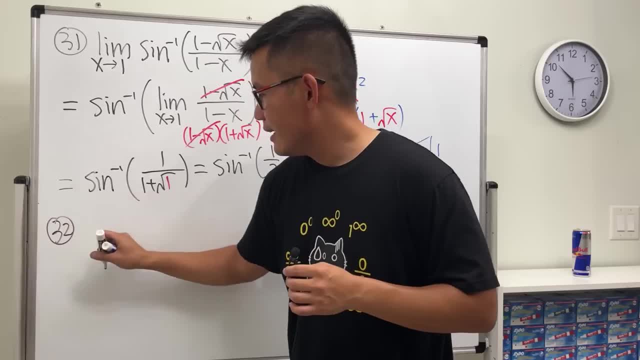 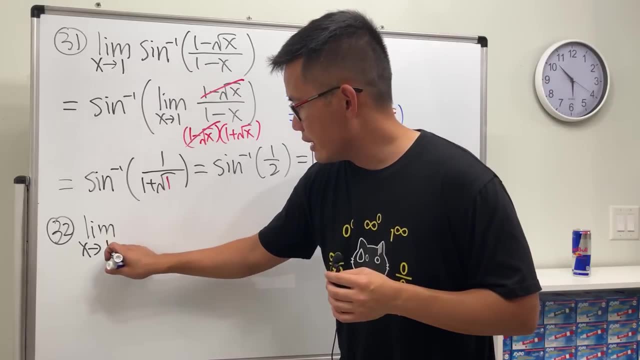 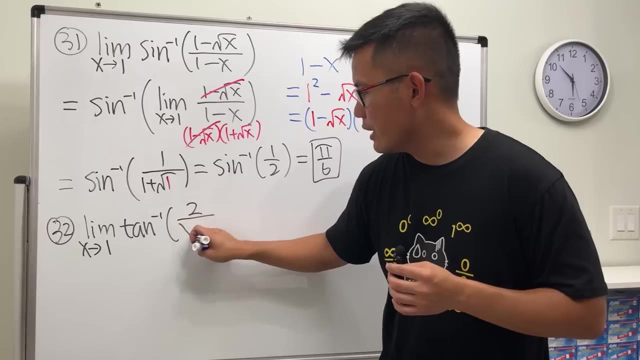 Next one, number 32.. All right, Here we have the limit as x approaching 1.. And then here I am going to give you guys inverse tangent of 2 over x minus 1.. Okay, Can we do the same that we did earlier? 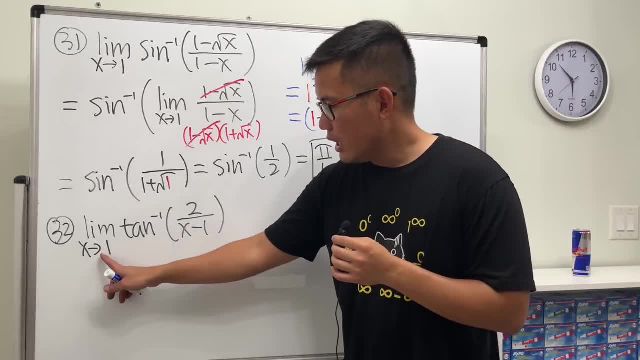 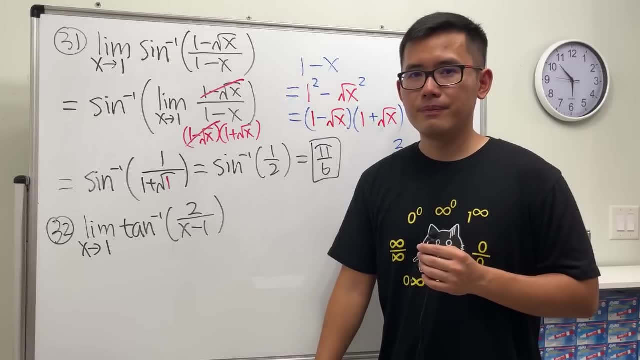 Not really. Not really in the following sense: because you see, if we put 1 inside here, we get 2.. We get 2 over 0.. Is it positive infinity or is it negative infinity? We will have to do what, Yeah. 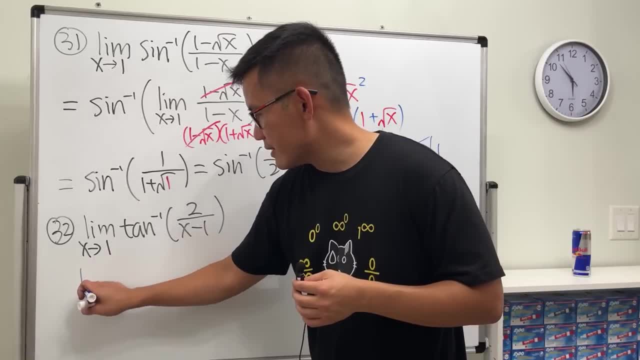 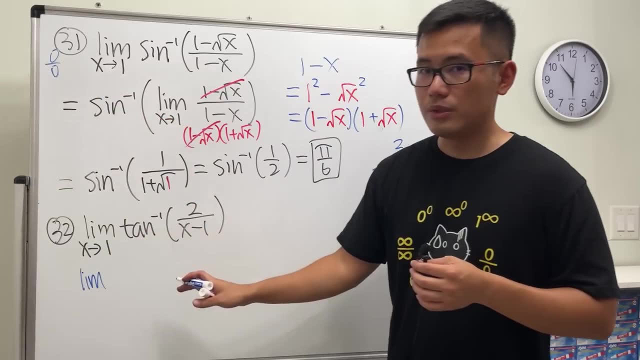 We will have to consider cases right. So let's break it down. This is not 0 over 0. This was 0 over 0. Let me just put it down somewhere. But this is not 0 over 0.. 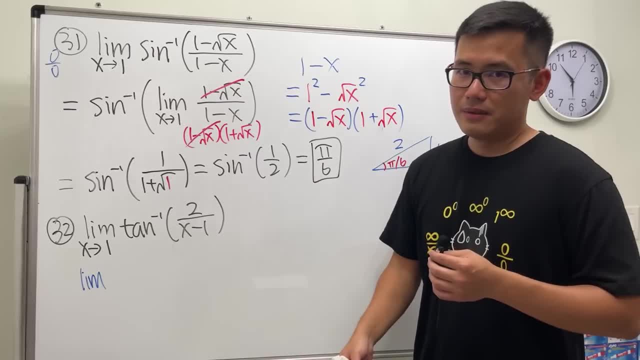 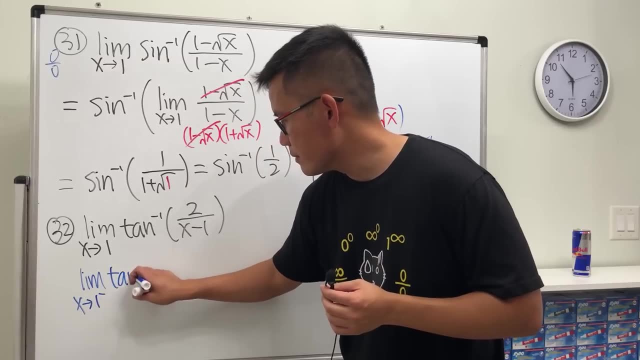 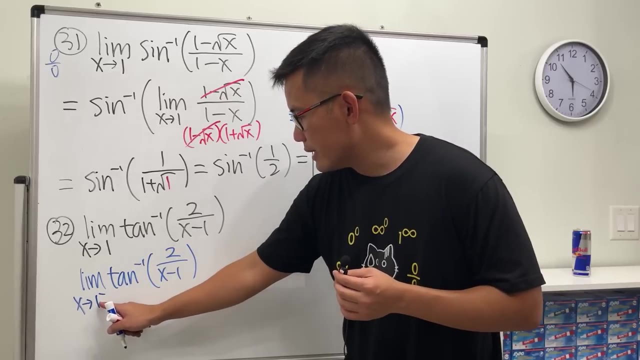 This is 2 over 0. So we have to do what we did like 2 hours ago, Anyway: x approaching 1 minus first. So what exactly do we get, though, If we do 1 minus? we put it here. 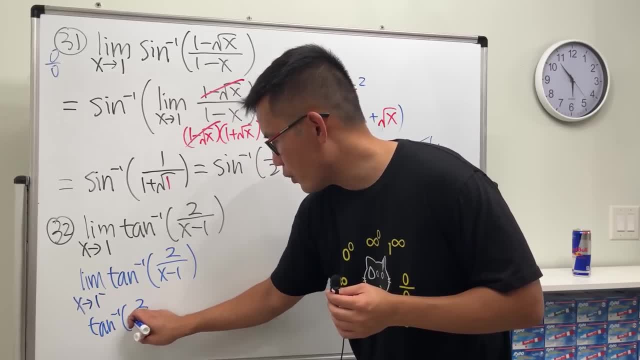 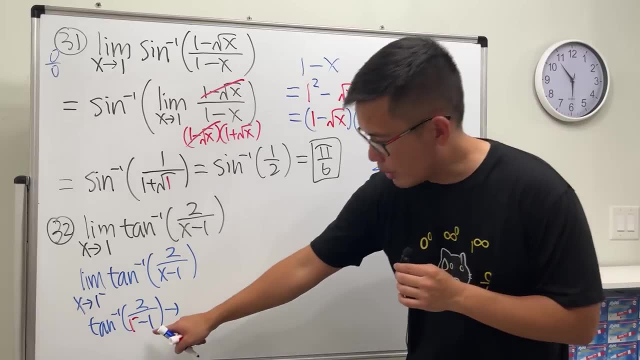 So we are looking at inverse tangent of 2 over, 1 minus and then minus 1.. So this is approaching what 1 minus 1 is 0, but this is 1 minus, So it's 0 minus right. 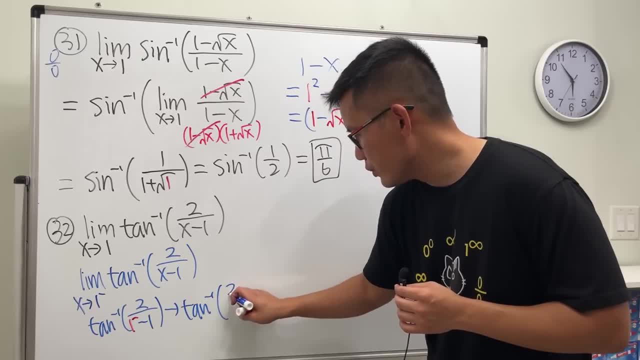 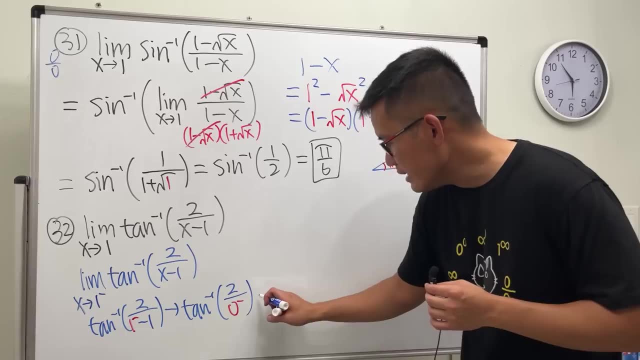 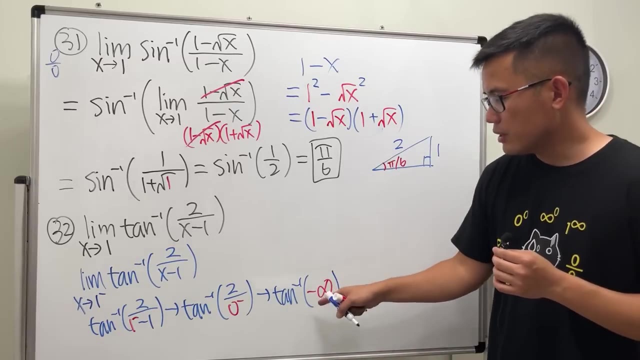 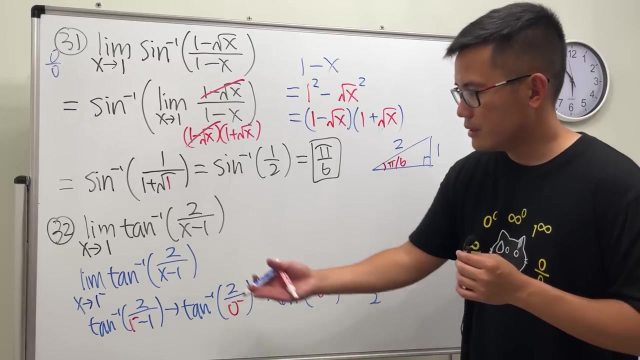 So this is inverse tangent of 2 over 0 minus 2 is positive, 0 minus is negative. So the inside will approach negative infinity. So inverse tangent of negative infinity is what This will approach negative pi over 2.. So this right here gives us negative pi over 2.. 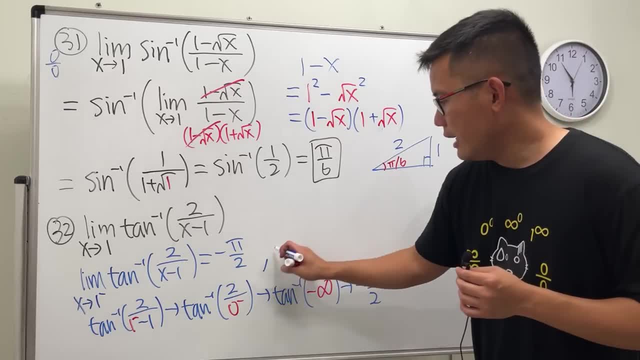 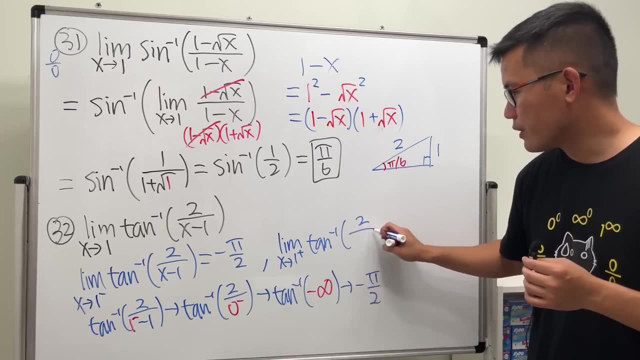 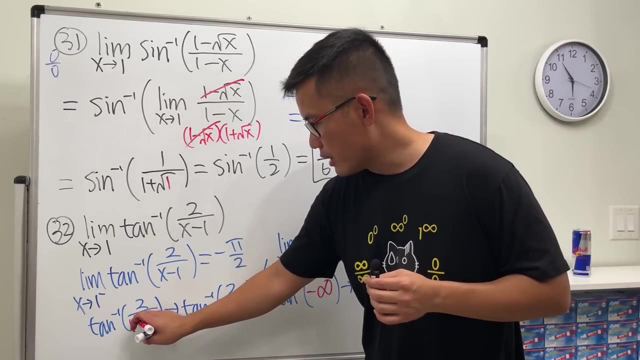 All right, Okay, And let's see If we have the limit as x approaching 1 plus inverse tangent of 2 over 1 minus 2 over x minus 1.. Well, you can see, I'm just going to change this right here. 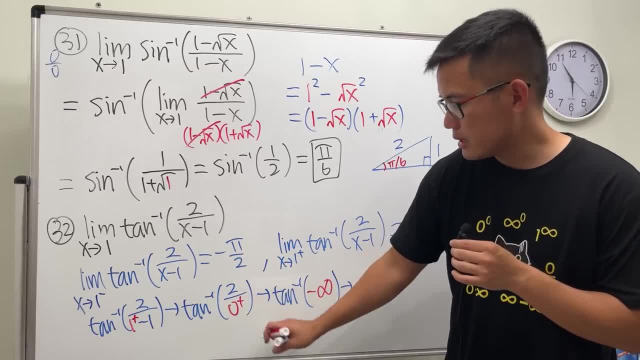 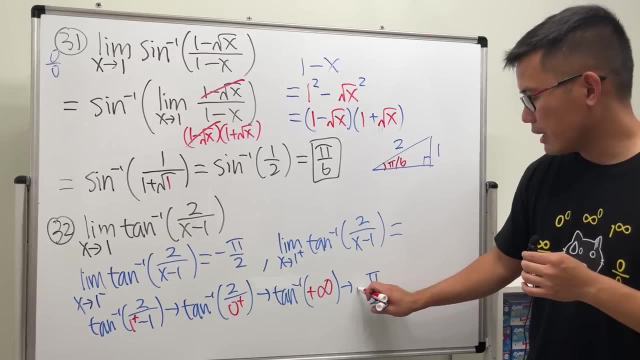 This is going to be 1 plus 1 plus minus 1 is 0 plus 2 over 0. plus is positive infinity, And then inverse tangent of positive infinity is positive pi over 2.. So this right here gives us positive pi over 2.. 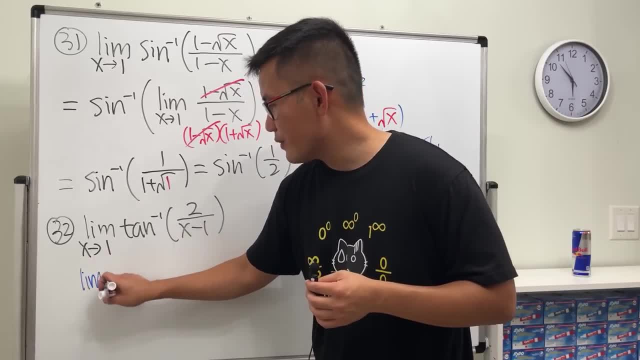 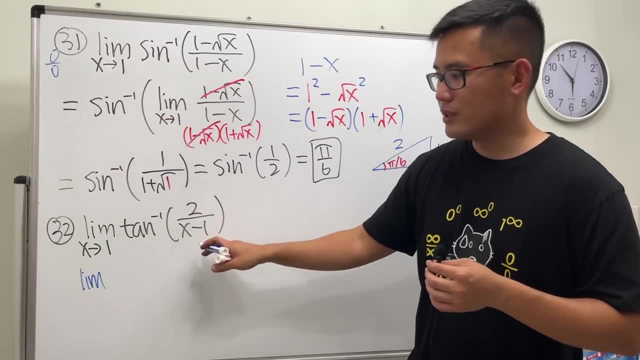 cases, right, so let's break it down. this is not 0 over 0, this was 0 over 0. let me just put it down somewhere. but this is not 0 over 0, this is 2 over 0. so we have to do what we did, like 2 hours ago anyway, X. 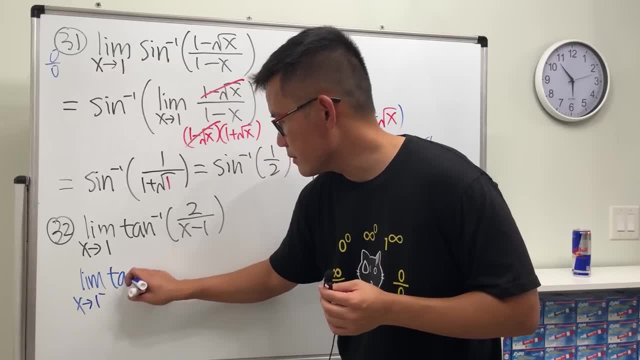 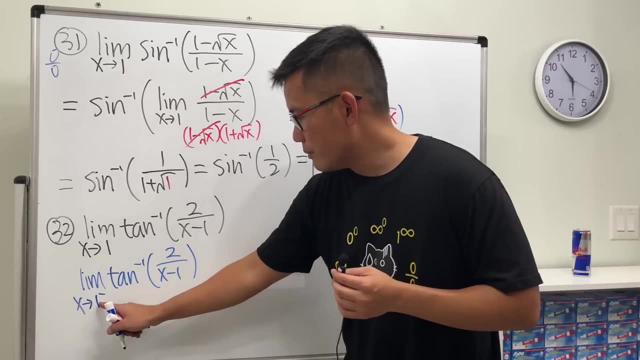 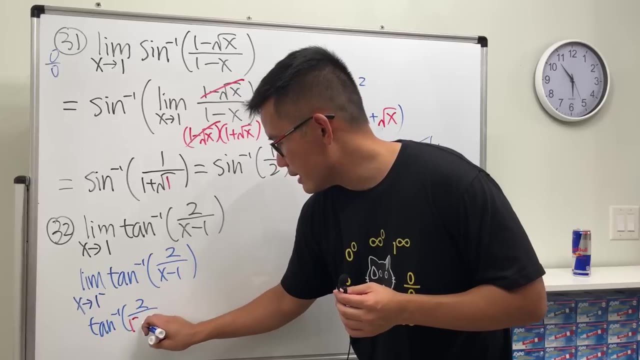 approaching 1 minus first. so what exactly do we get? oh, if we do 1 minus, we put it here. so we're looking at inverse tangent of 2 over, 1 minus and then minus 1. so this is approaching what? 1 minus 1 is 0, but this is 1 minus. 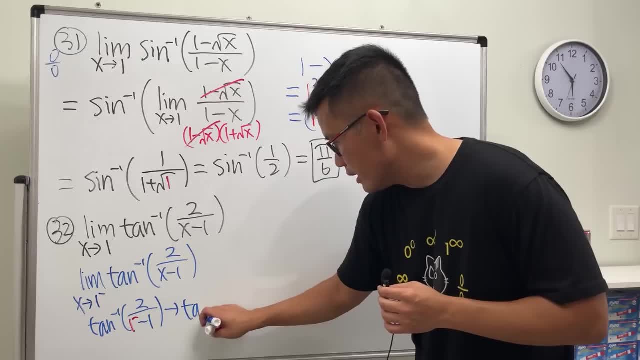 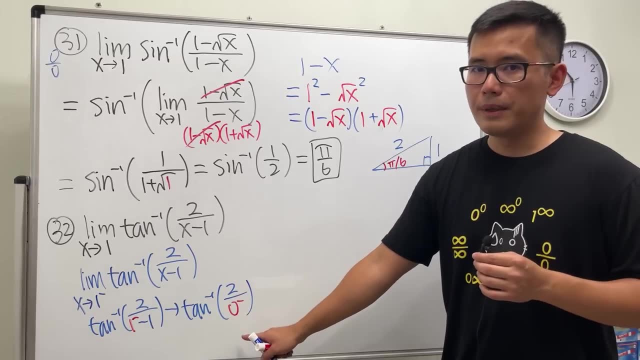 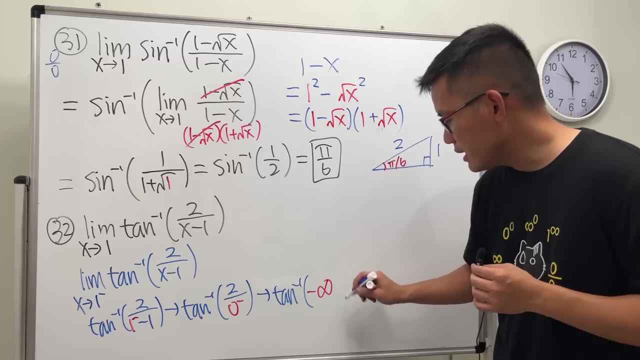 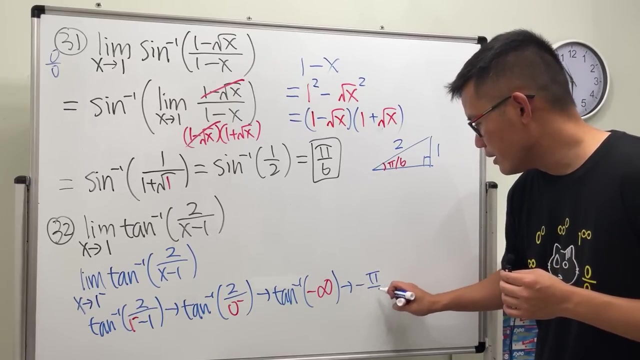 so it's 0 minus right. so this is inverse tangent of 2 over 0 minus 2 is positive, 0 minus is negative. so the inside will approach in the negative infinity. so inverse tangent of negative infinity is what this will approach: negative pi over 2. so this right here gives us negative pi. 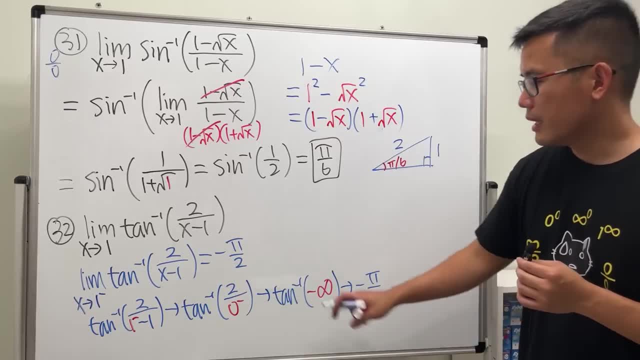 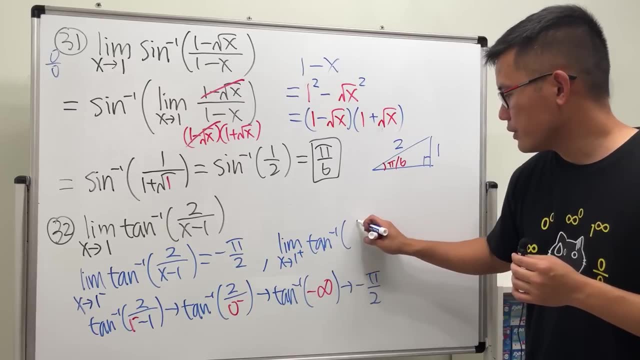 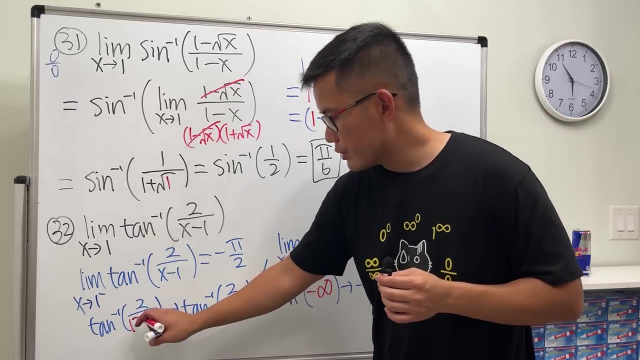 over 2. All right, okay, and let's see if we have the limit as x approaching 1 plus inverse tangent of 2 over x minus 1.. Well, you can see, I'm just going to change this right here. This is going to be 1 plus. 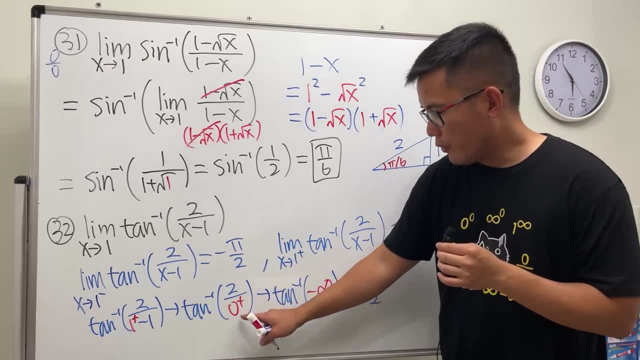 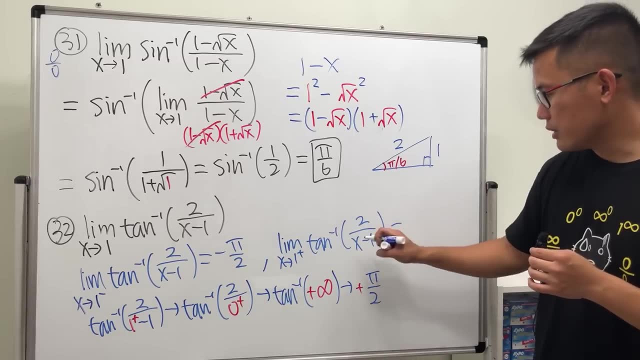 1 plus minus 1 is 0 plus 2 over 0 plus is positive infinity, and then inverse tangent of positive infinity is positive pi over 2.. So this right here gives us positive pi over 2.. Unfortunately they are not the same. 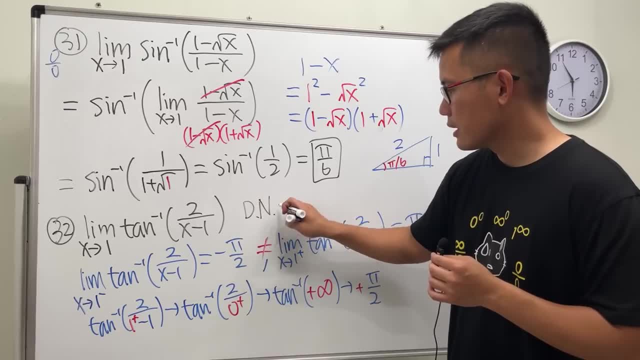 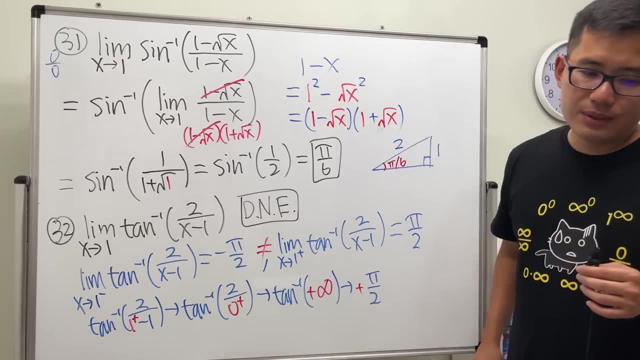 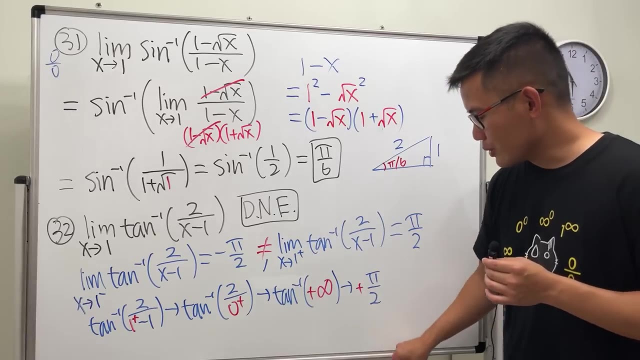 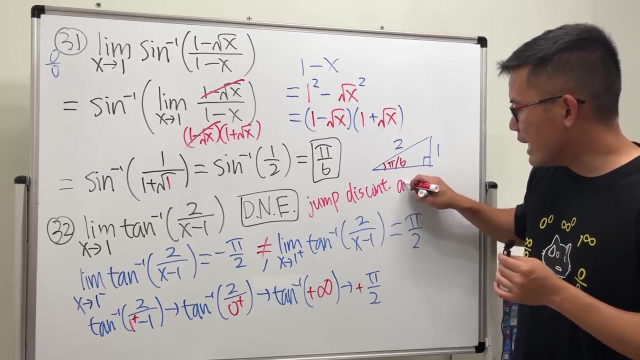 Therefore, this limit does not exist And, in fact, in this particular case- I don't remember I forgot to mention this earlier- In this particular case we actually have a so-called jump, This, This continuity at x equal to 1.. 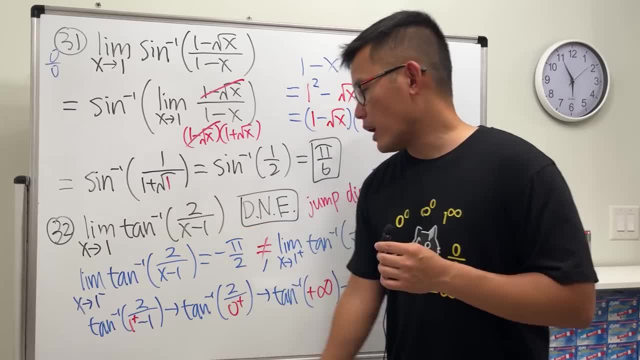 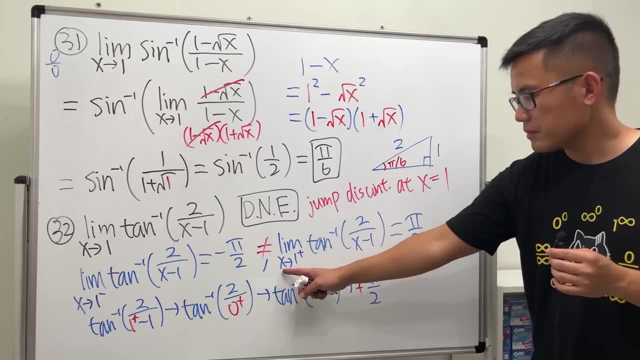 Why? Because, as you can see, when x is approaching 1 from the left-hand side, it does have a limit, But that limit is not the same as when we approach the 1 from the right-hand side. These two limits have to be finite. 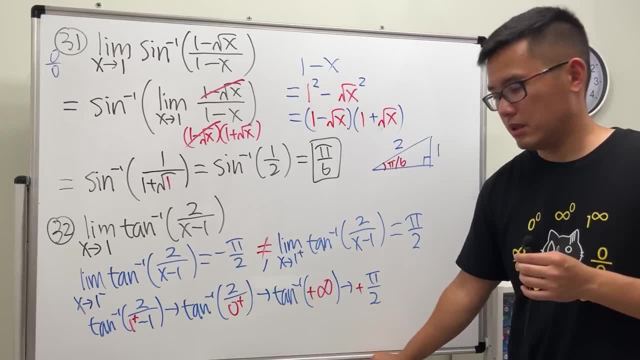 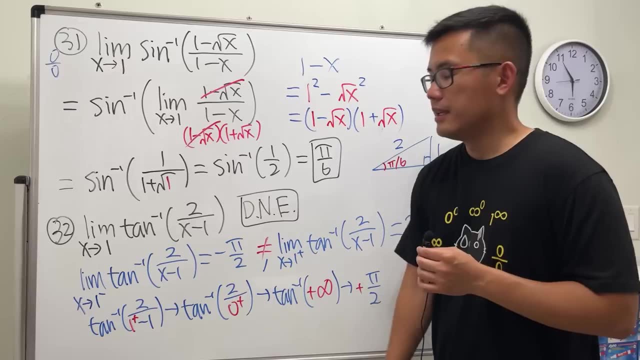 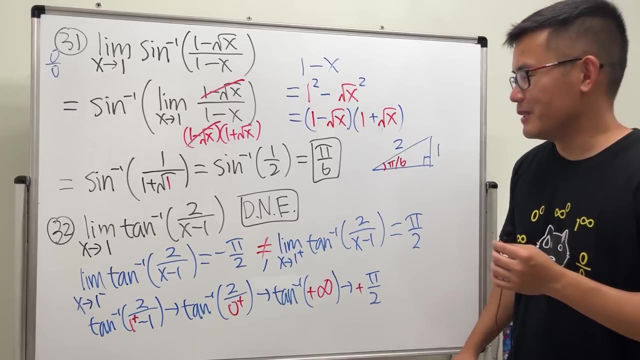 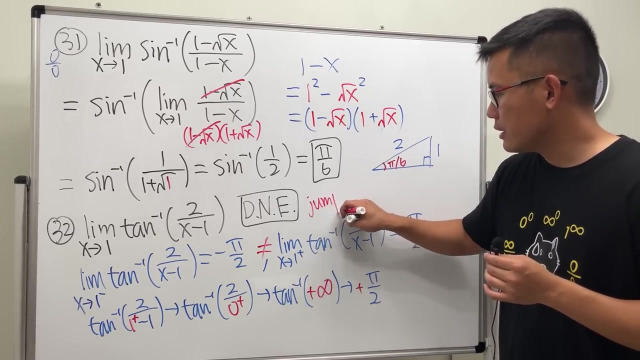 Unfortunately, they are not the same. Therefore, this limit does not exist And, in fact, in this particular case- I don't remember I forgot to mention this earlier- In this particular case we actually have a so-called jump. 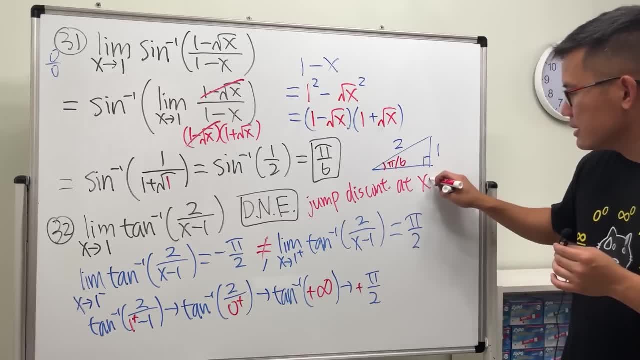 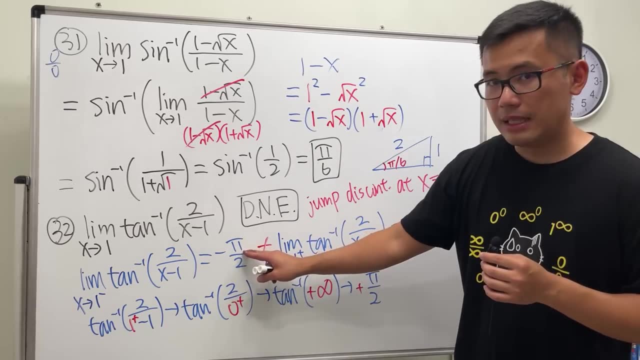 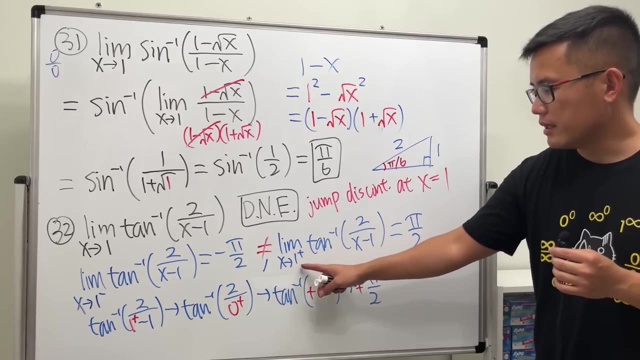 This continuity at x equal to 1.. Why? Because, as you can see, when x is approaching 1 from the left-hand side, it does have a limit, But that limit is not the same as when we approach the 1 from the right-hand side. 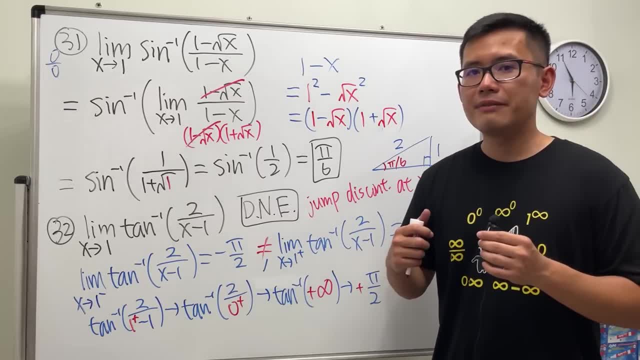 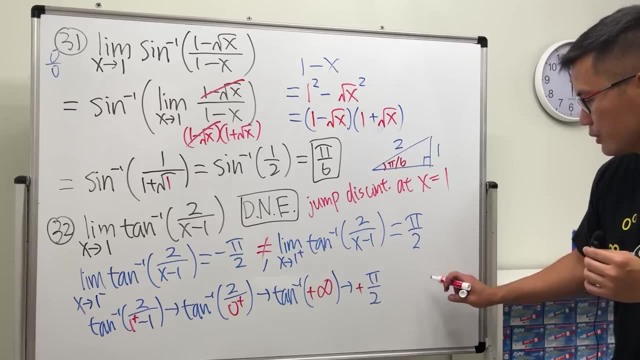 These two limits have to be finite And they have to be different to invert for us to have a jump, this continuity. The picture of this should look like the following. I'll just give you guys a picture real quick. 1 is right here. 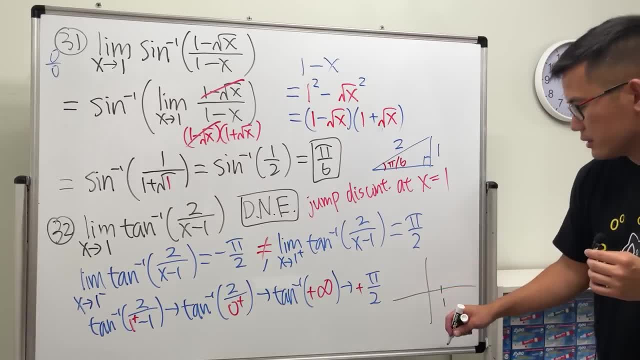 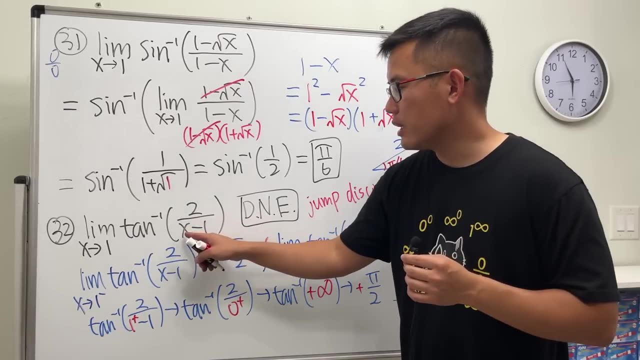 When x is approaching 1, negative, it's negative pi over 2, right, So you will get. And when x is in negative infinity, we get 0.. So, yeah, you'll get like this, And then negative pi over 2.. 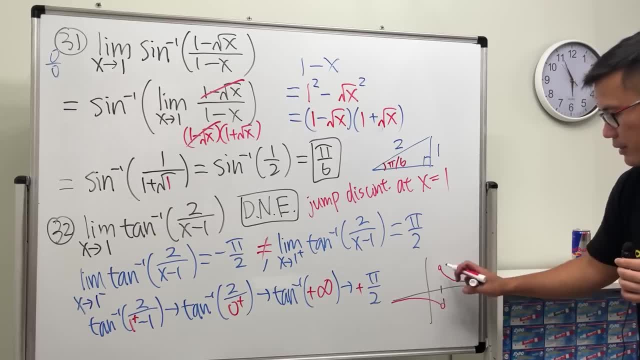 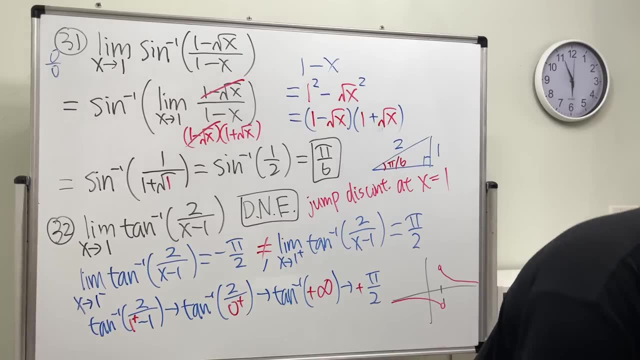 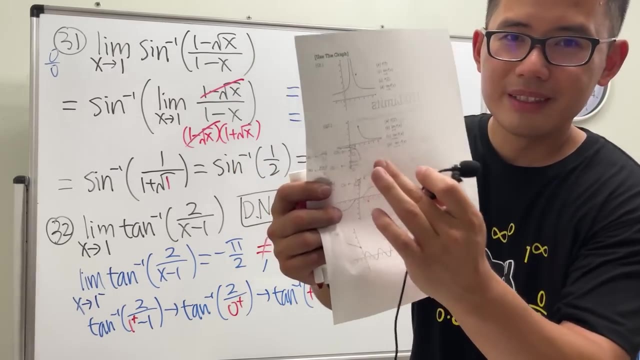 And then like this: Yeah, so there's a jump. It's very similar to: Oh man, yes, It's actually question number 2.. There's a jump right here too. There's a jump When x is at 2, right there. 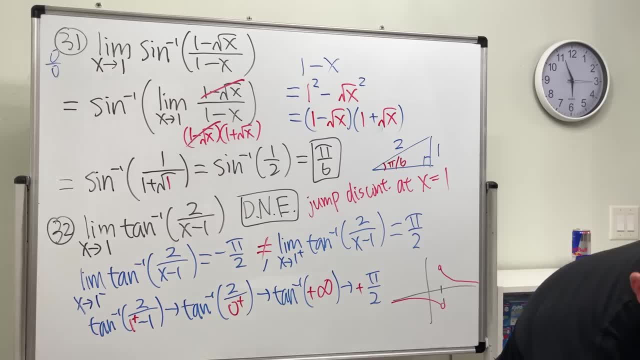 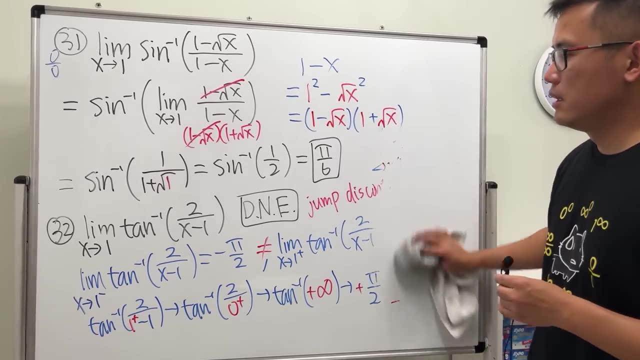 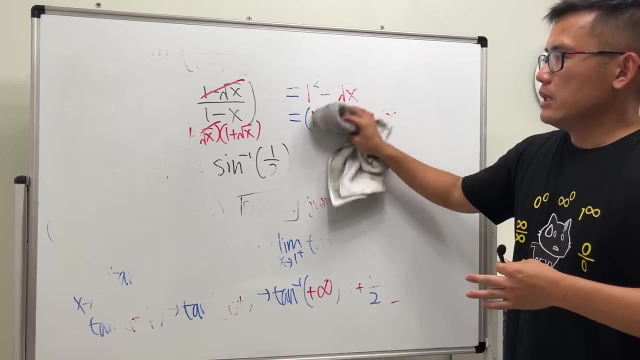 So yeah, I forgot to mention it. Anyway, That's number 32.. So sometimes when x is approaching to some number, you don't have to do. You may not get 3 over 0, but if you get like 2 over 0,. 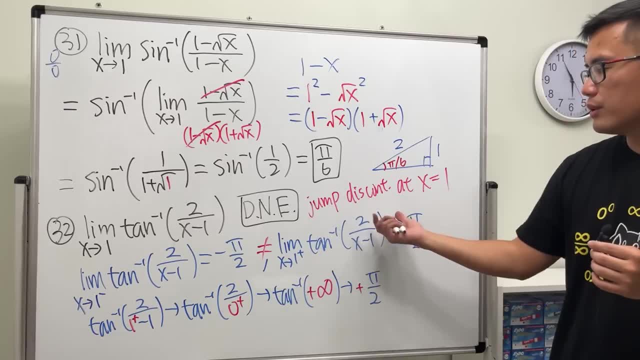 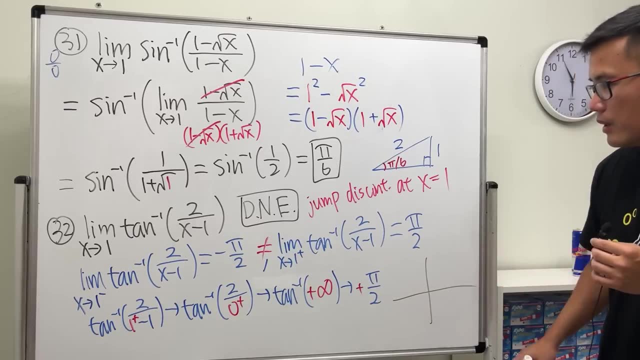 and they have to be different to invert for us to have a jump discontinuity. The picture of this should look like the following: So you know, just to give you guys a picture real quick, 1 is right here. When x is approaching 1 negative, it's negative. pi over 2, right. 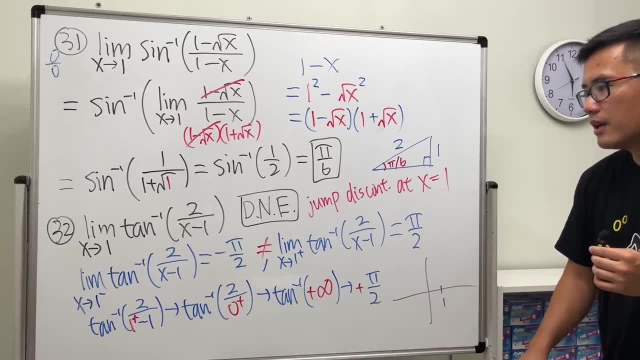 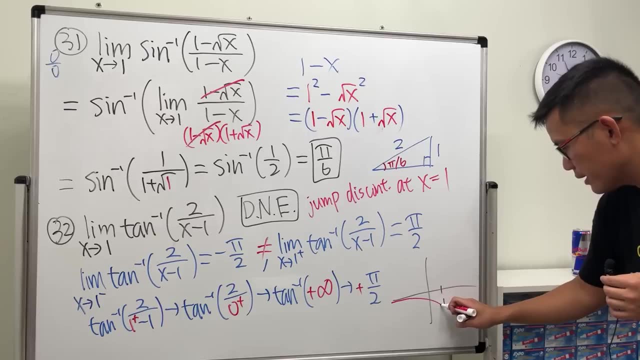 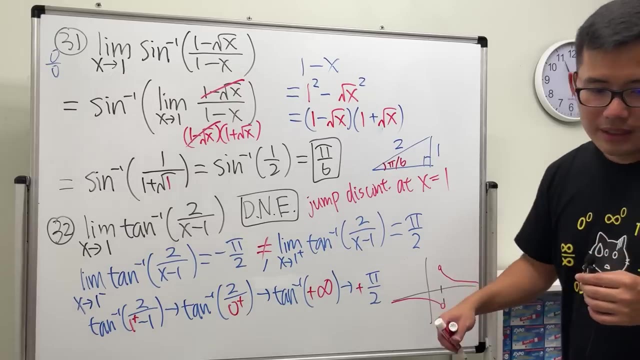 So you will get, And when x is in negative infinity, we get 0.. So, yeah, you'll get like this, And then negative pi over 2. And then like this: Yeah, so there's a jump. It's very similar to. 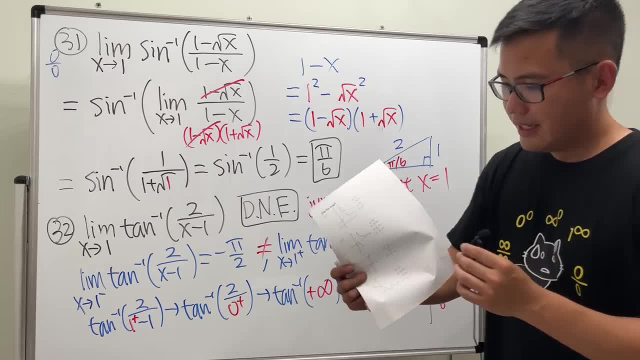 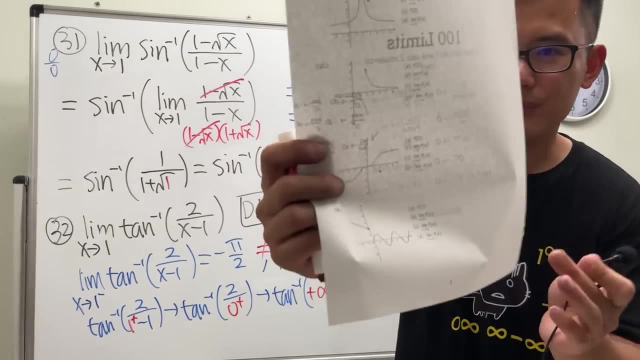 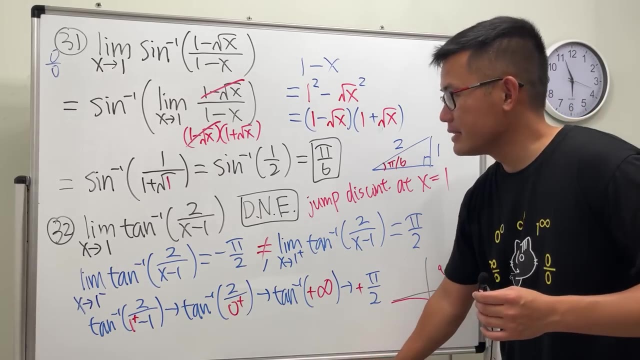 Oh man, yes, It's actually question number 2.. There's a jump right here too. There's a jump When x is at 2, right there. So yeah, I forgot to mention it. Anyway, That's number 32.. 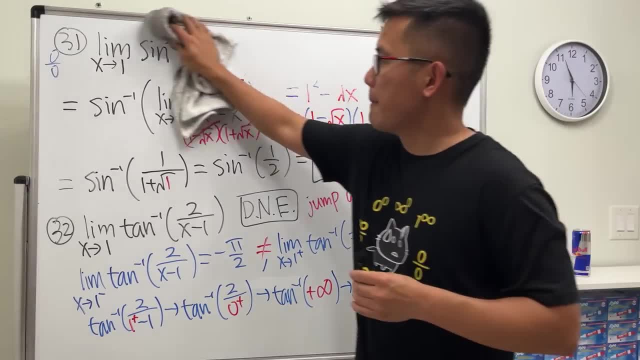 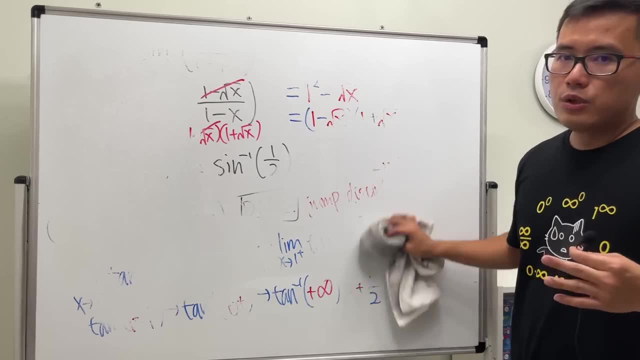 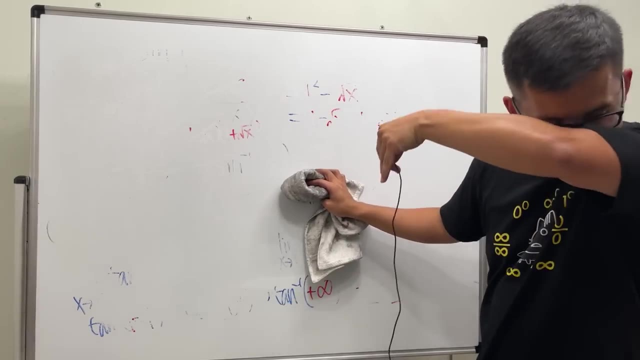 Number 32.. So sometimes, when x is approaching to some number, you don't have to do. You may not get Look for a zero, But if you get like 2 over 0,, like 5 over 0, then break down into cases like the things that we did earlier. 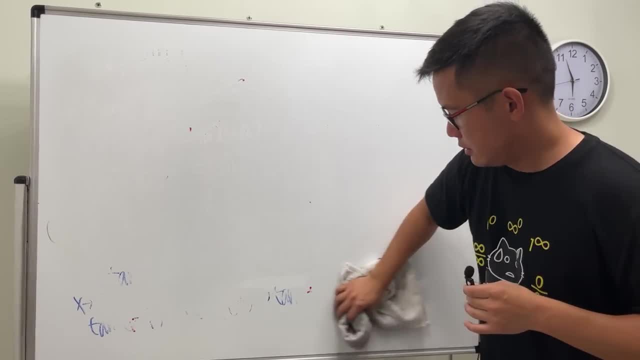 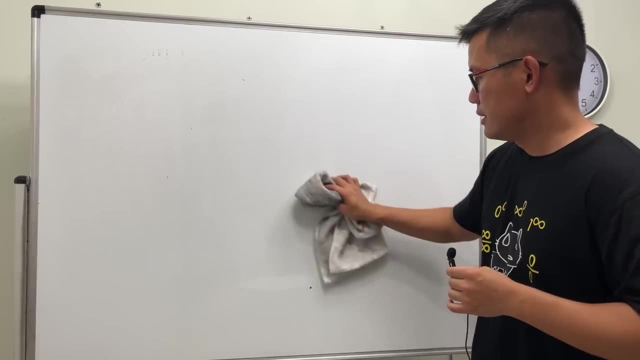 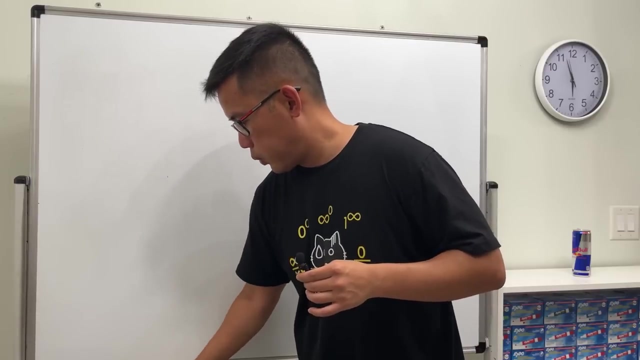 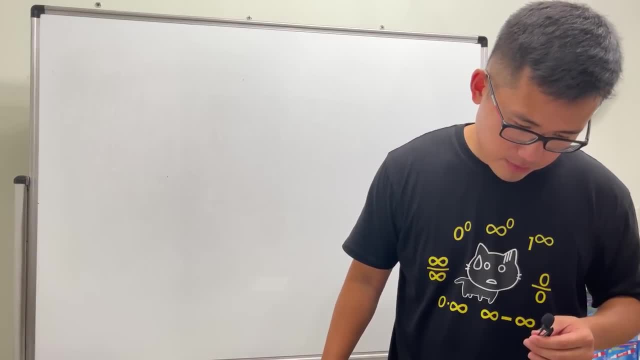 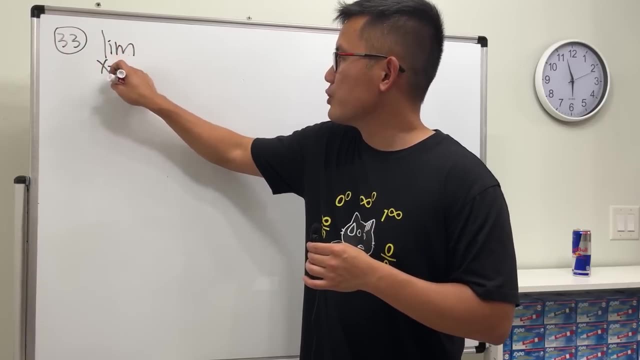 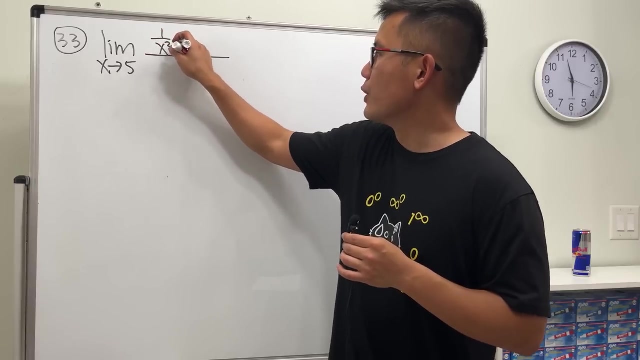 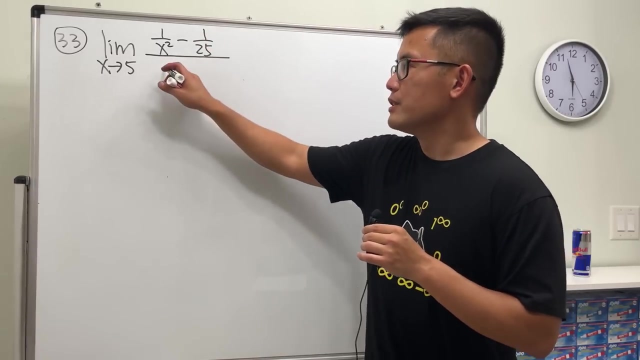 number 33 here, limit as x approaching 5. and then we have 1 over x, squared minus 25, so 1 over x, squared minus 1 over 25. i forgot what i said. and then on the bottom we have x minus. sorry, we have x squared minus 25. 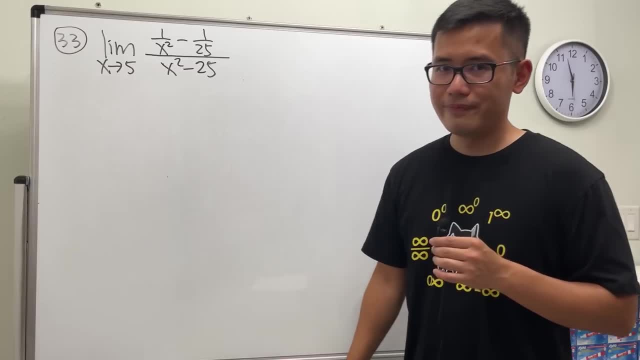 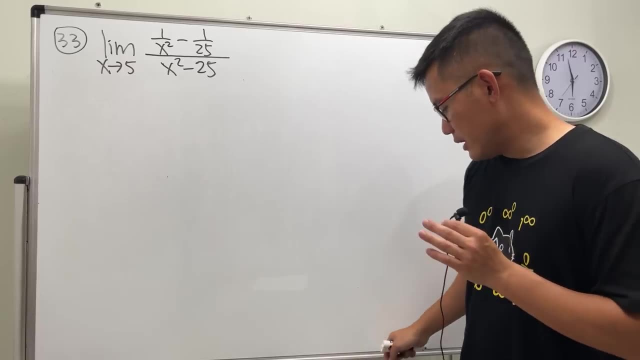 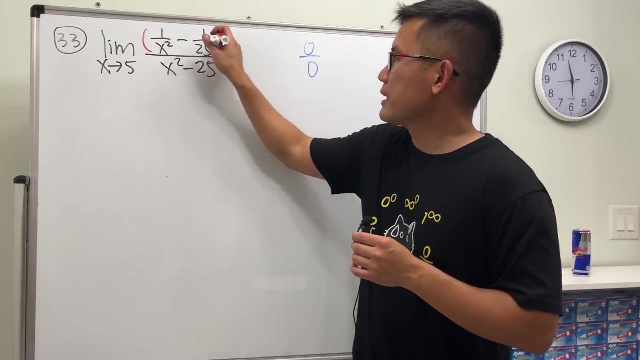 cool- do not cancel this- and that they are very different. fix the complex fraction first, and, yes, this is a zero over zero situation. okay, check it real quick. by the way, though, let's multiply the top and bottom by this and that which is 25 x squared. 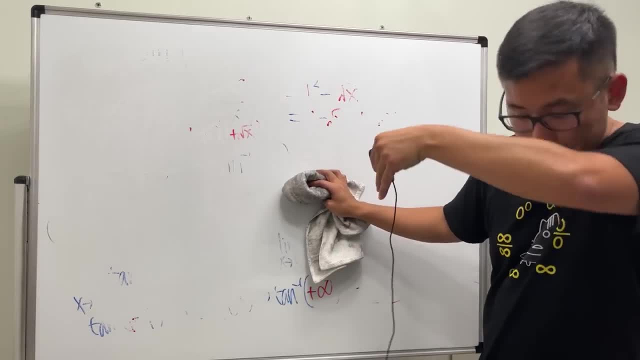 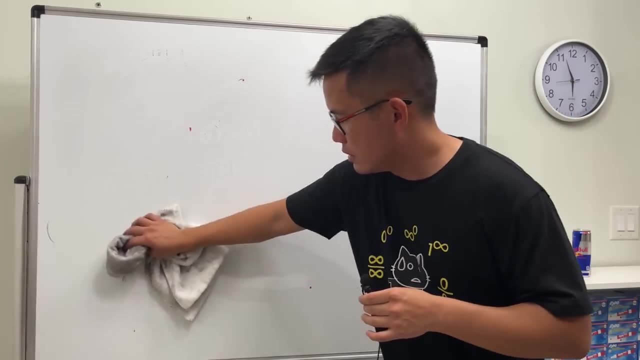 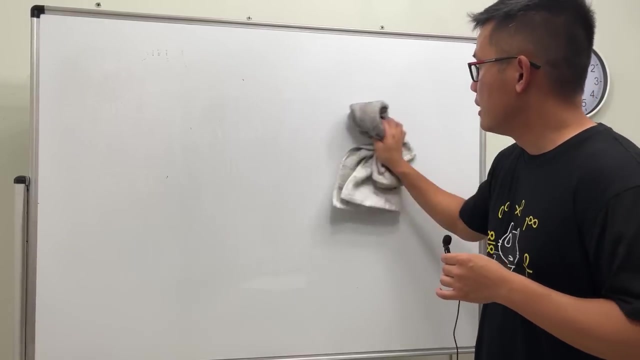 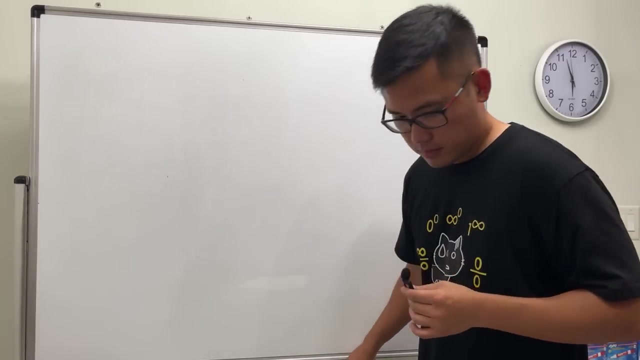 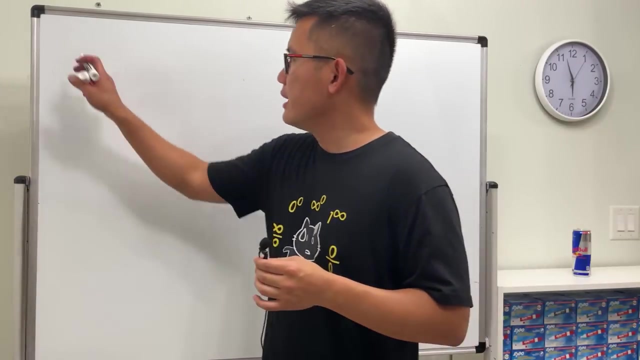 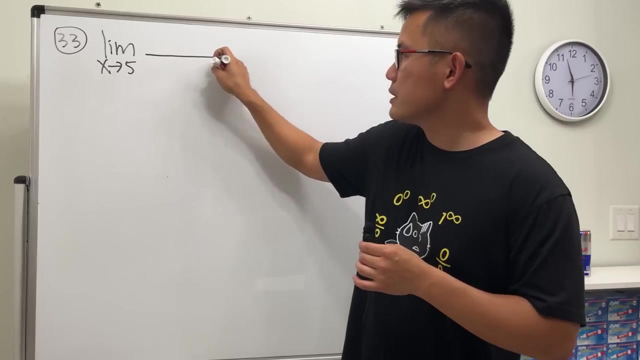 like 5 over 0,. you can break down into cases like the things that we did earlier, So those will be helpful. Number 33. Here limit as x approaching 5.. And then we have 1 over x, squared minus 25.. 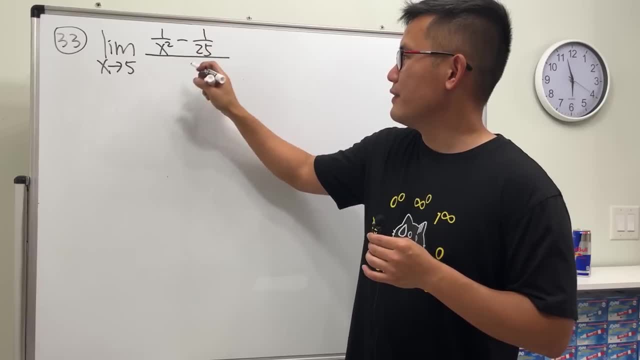 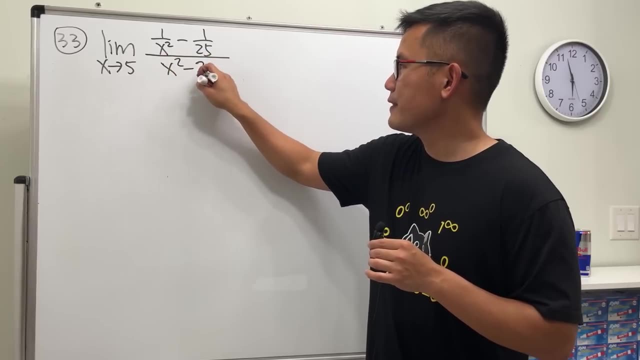 So 1 over x squared minus 1 over 25.. I forgot what I said. And then on the bottom, we have x minus. Sorry, we have x squared minus 25.. Cool, Do not cancel this. and that They are very different. 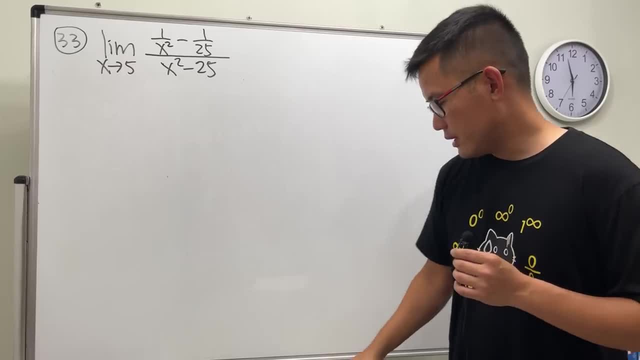 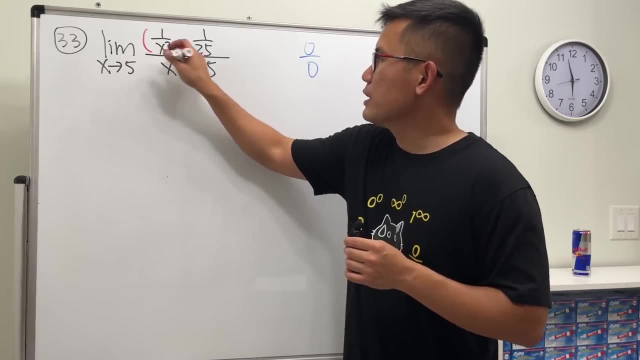 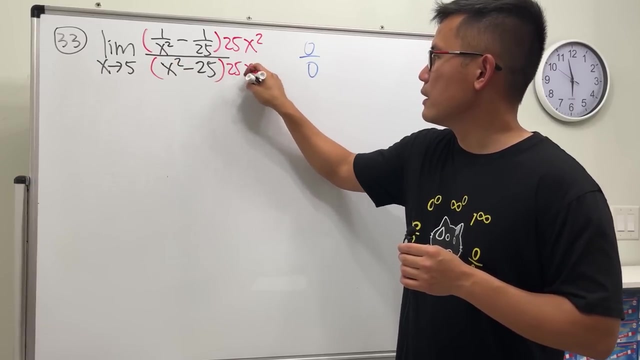 Fix the complex fraction first, And yes, this is a 0 over 0 situation. Check it real quick. By the way, though, let's multiply the top and bottom by this and that which is 25x squared, So we are going to get 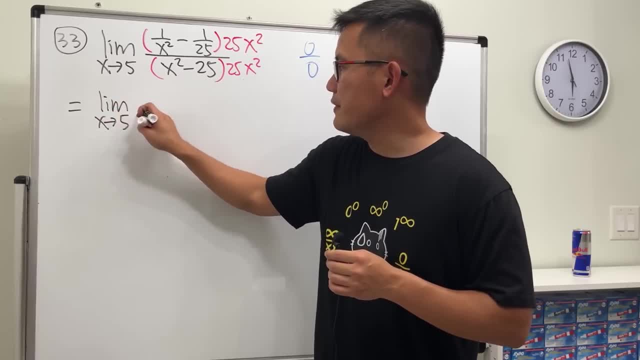 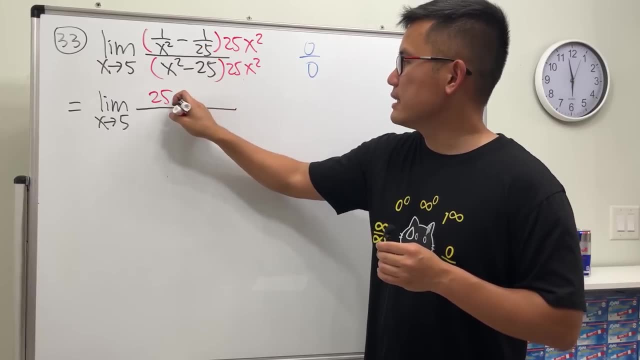 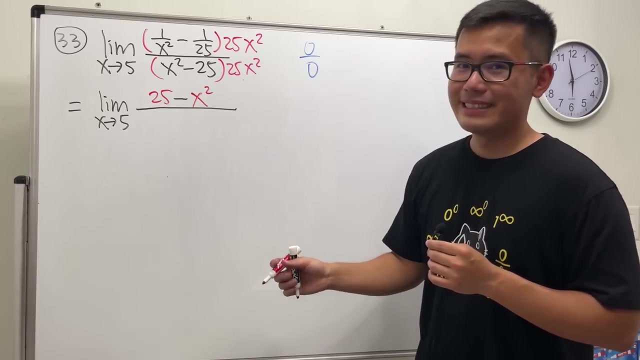 the limit as x approaching 5.. This times that the x squared will cancel, so we get 25.. Minus This times that the 25 will cancel, so we have 25 minus x squared On the bottom. you guessed it. 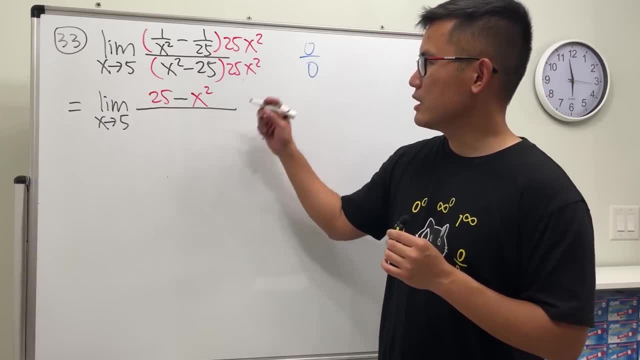 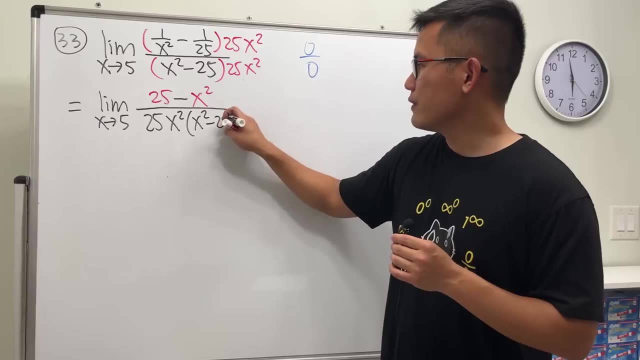 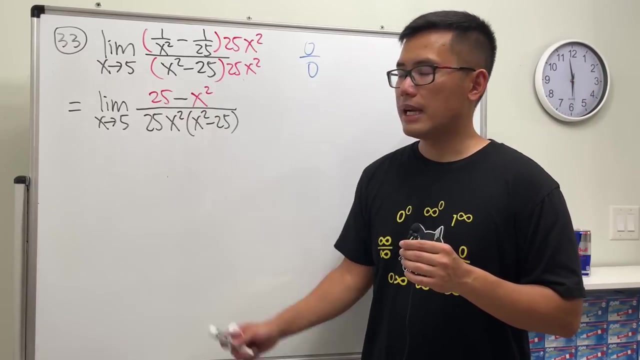 we are not going to multiply things out. Let's just keep it as how it is: 25x squared times x squared minus 25.. Yeah, cool, Now can we cancel this and that? No, not yet. This is kind of out of order. 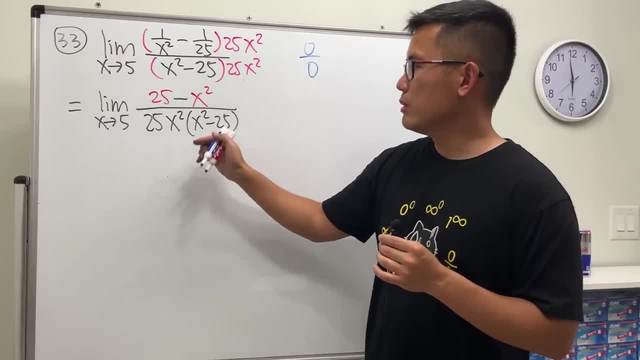 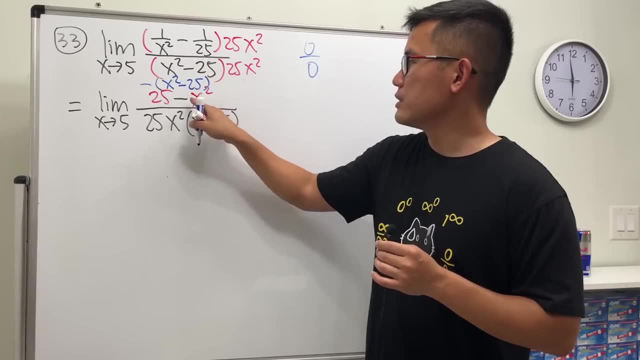 We'd like to have the x squared goes first right, And we can do so by just changing right factorial or negative, and then we can say: this is x squared minus 25.. So this and that are the same. Now we can cancel the x squared minus 25.. 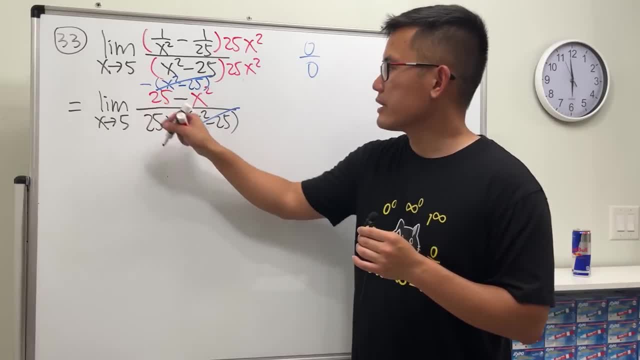 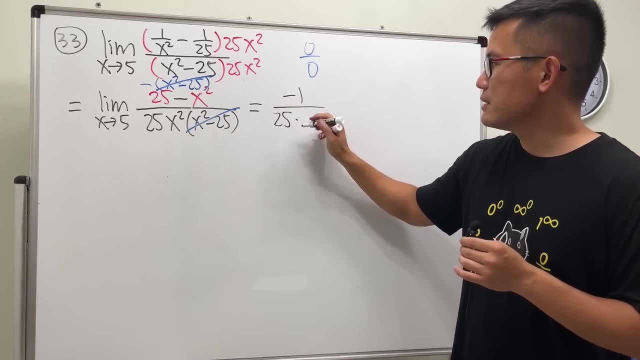 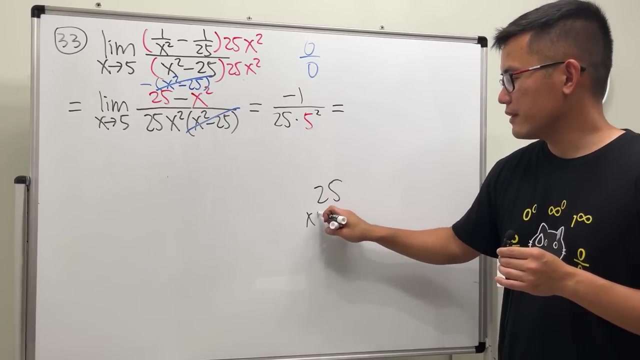 Yeah. So what do we have On the top? we still have the negative, And it's a negative 1. On the bottom we have this: 25. Times 5 squared, which is just 25.. So what's 25 times 25?? 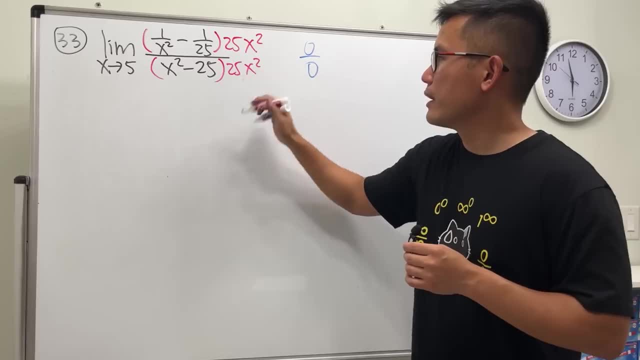 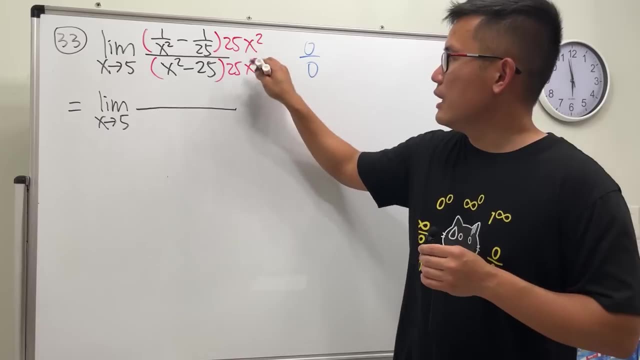 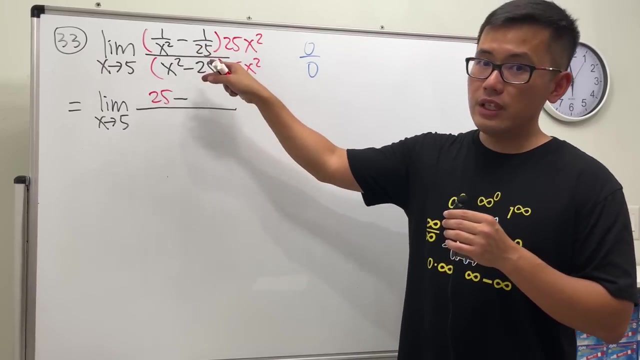 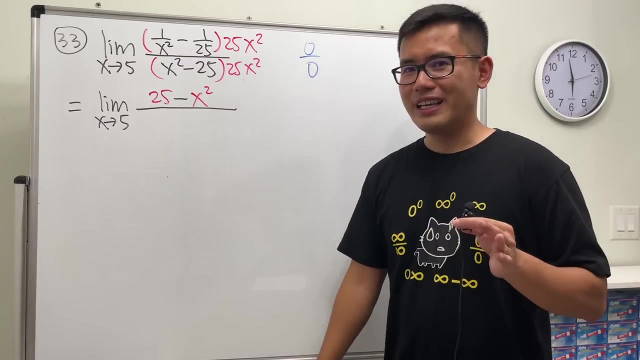 so we are going to get the limit as x approaching 5. this times that the x squared will cancel. so we get 25 minus this times that the 25 will cancel. so we have x. we have 25 minus x squared on the bottom. you guessed it. we are not going to cancel things. 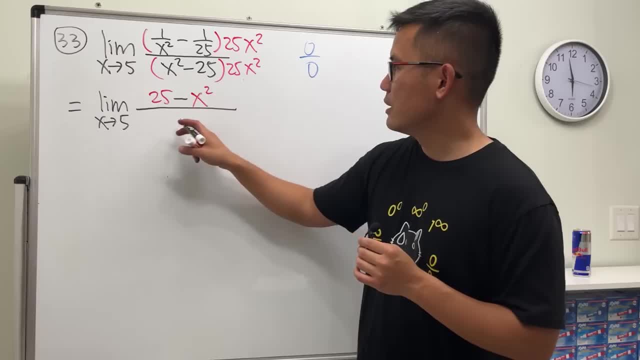 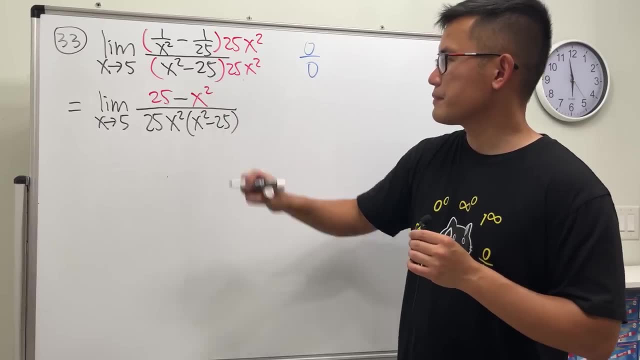 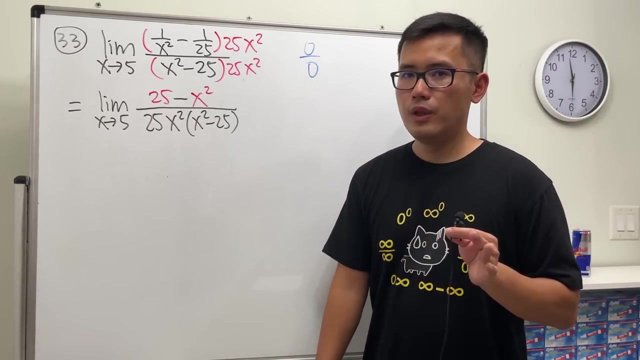 we are not going to multiply things out, let's just keep it as how it is: 25 x squared times x squared minus 25. yeah, cool, now can we cancel this and that? no, not yet this is kind of out of order. we like to have the x squared goes first, right. 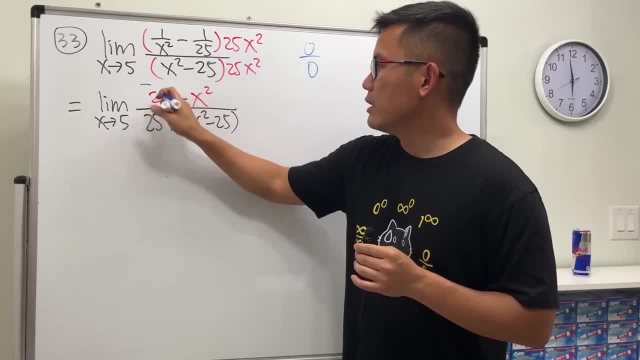 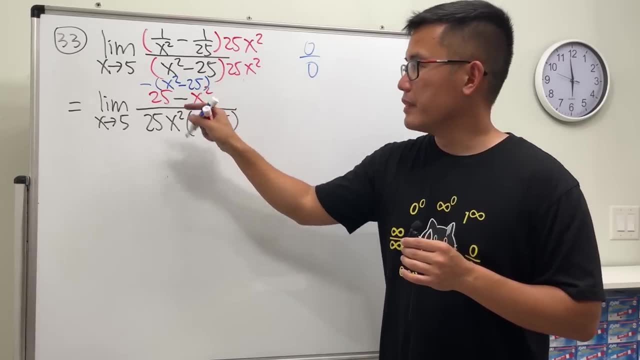 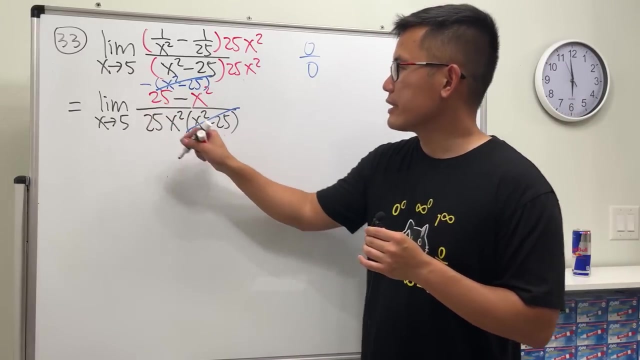 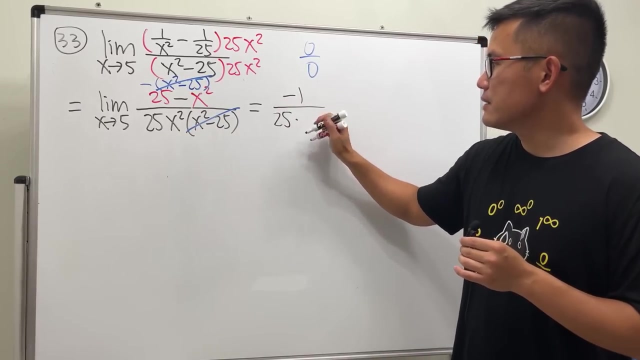 and we can do so by just changing right factorial negative, and then we can say: this is x squared minus 25. so this and that are the same. now we can cancel the x squared minus 25. yeah, so what do we have? on the top, we have a negative and it's a negative 1 on the bottom, we have this 25 times 5. 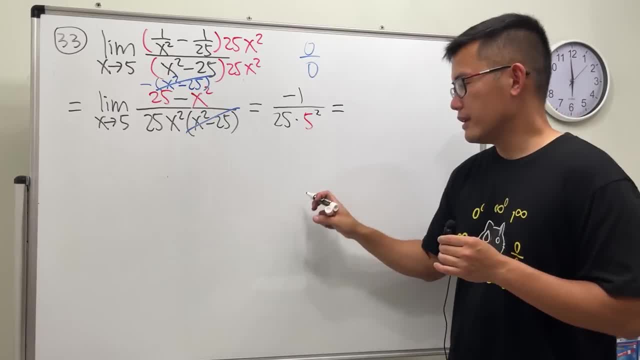 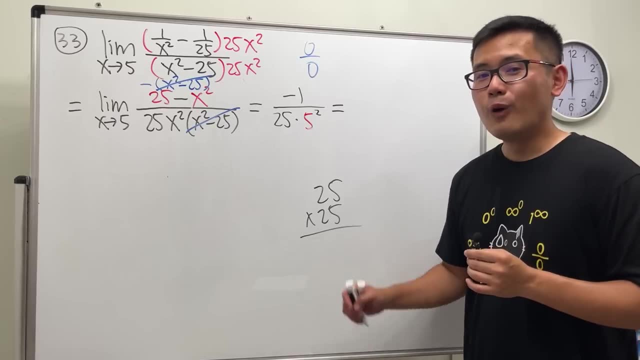 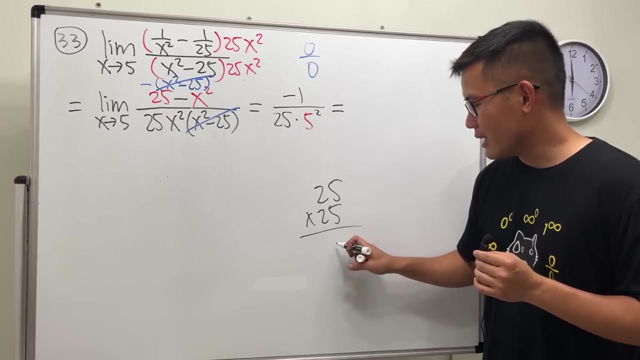 squared, which is just 25. so what's 25 times 25? I want to show you guys the best way to do it. whenever you are multiplying two numbers, if they end with a 5, yeah, you can do the following: 5 times 5 is what 25? okay, you do 2 times 5. 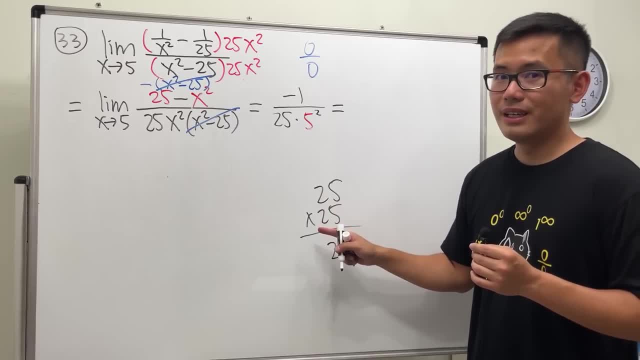 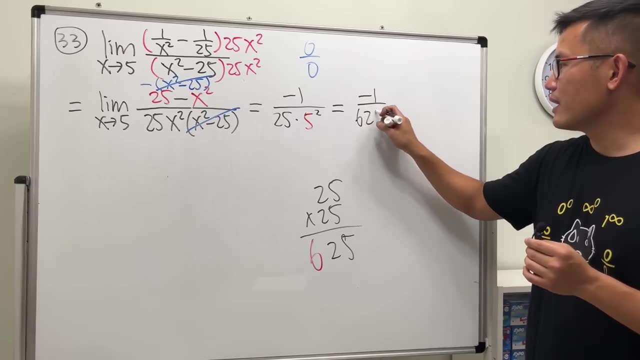 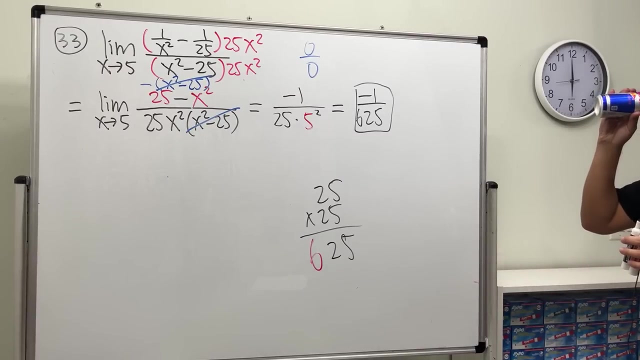 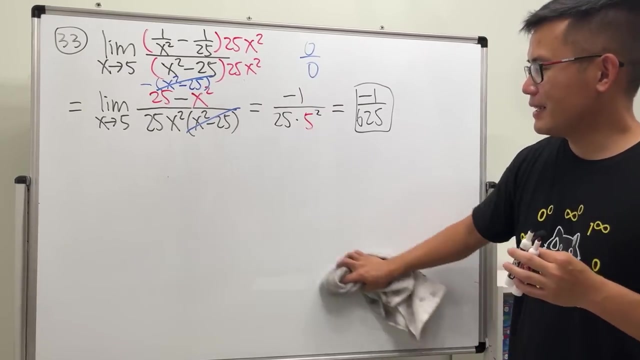 not 2, but times the next number, which is 3, 2 times 3 is 6, so 625. so it's negative 1 over 625. okay, I have a video on that- pretty cool stuff. you guys can go and check that out on my just algebra channel. 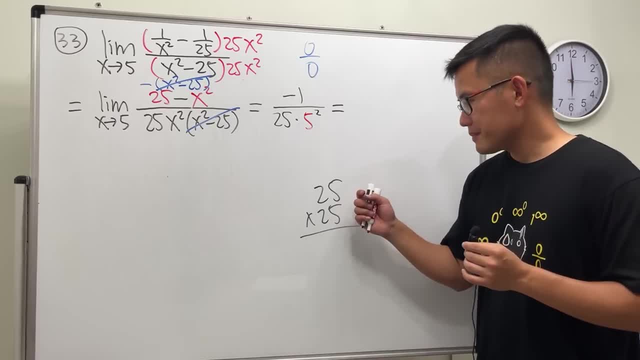 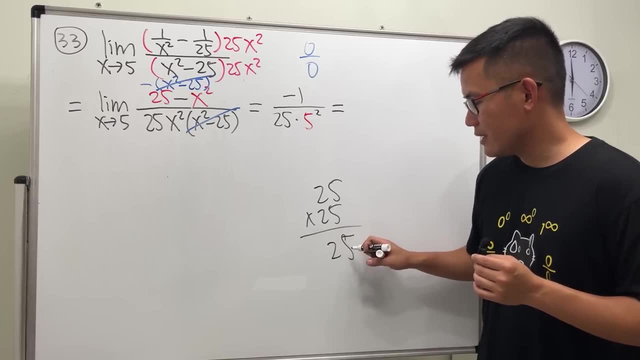 I want to show you guys the best way to do it. Whenever you are multiplying two numbers, if they end with a 5, you can do the following: 5 times: 5 is what 25.. Okay, You do 2 times. 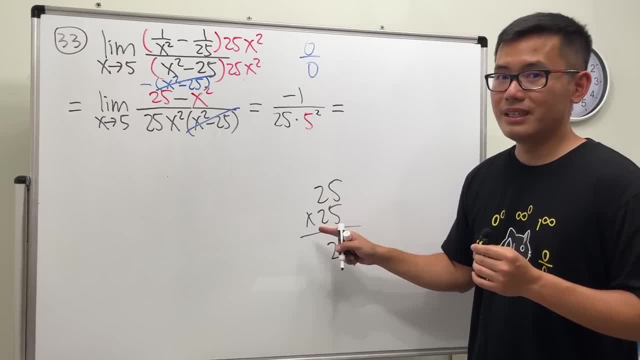 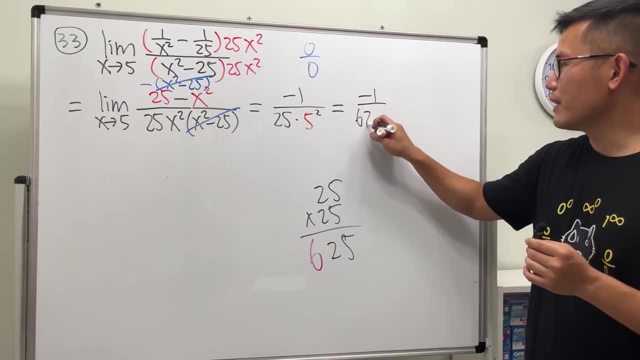 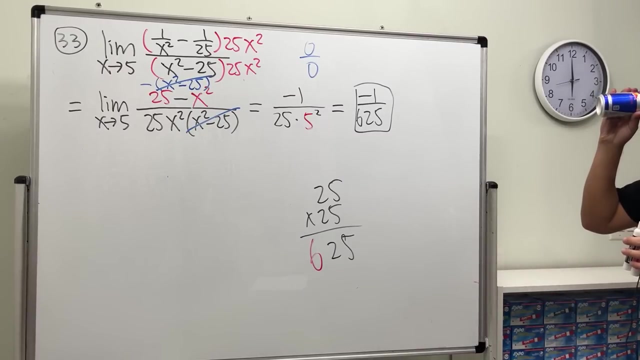 not 2, but times the next number, which is 3.. 2 times 3 is 6.. So 625.. So it's negative 1 over 625.. Okay, I have a video on that. Pretty cool stuff. 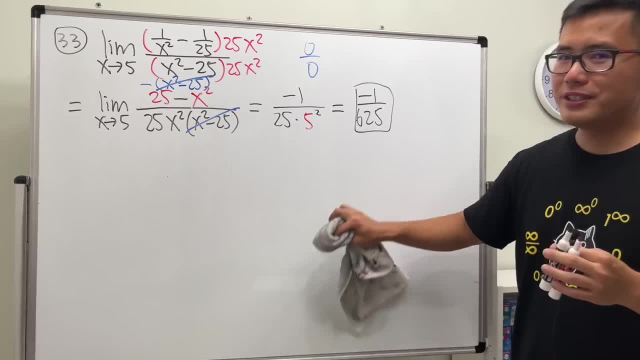 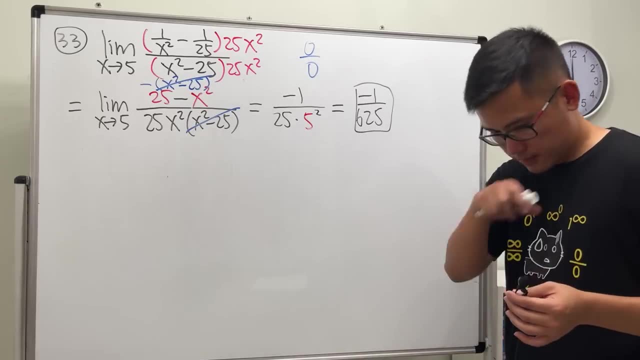 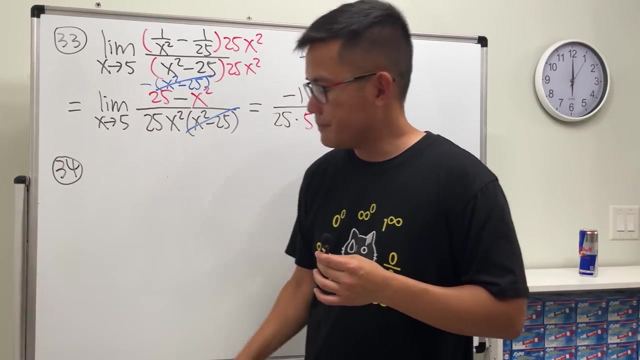 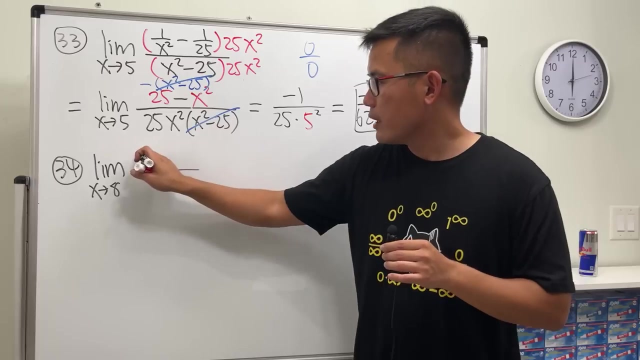 You guys can go and check that out on my Just Algebra channel. All right, Ladies and gentlemen. number 34. Limit as x approaching 8.. And then we have the cube root of x minus 2 over x minus 8.. Wow. 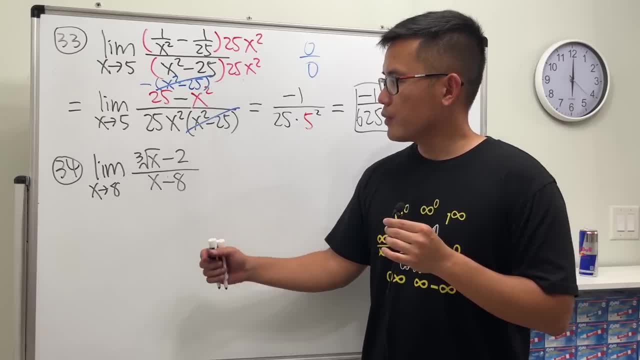 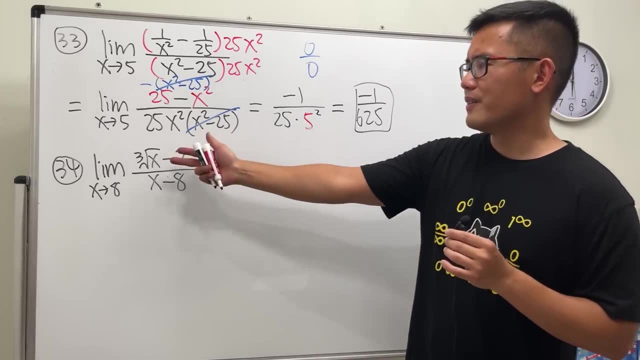 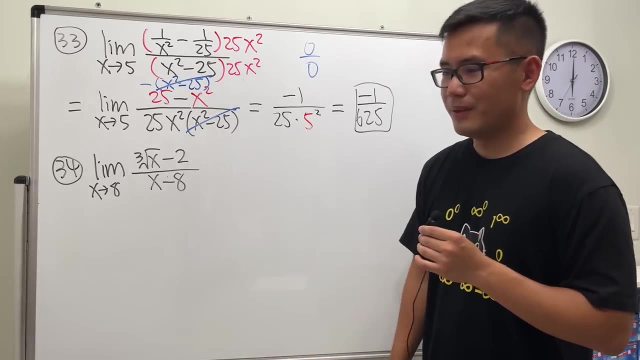 How do we do this? We can multiply by the conjugate to kind of complete the to get rid of the cube root. That's, that's possible. But let's look at the following. All right, Firstly, we can factor this: 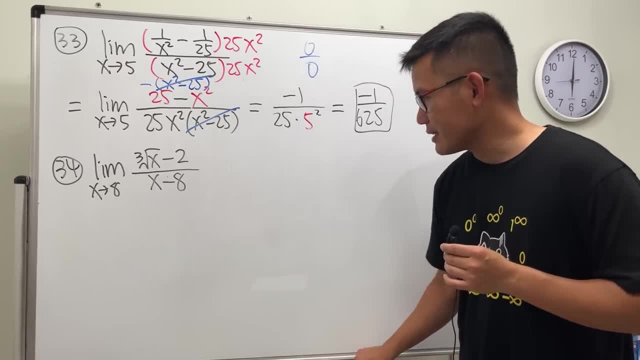 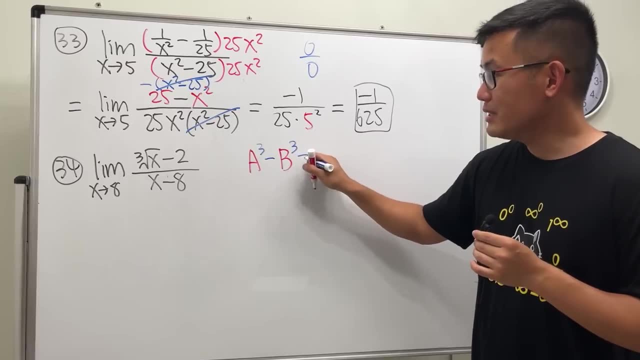 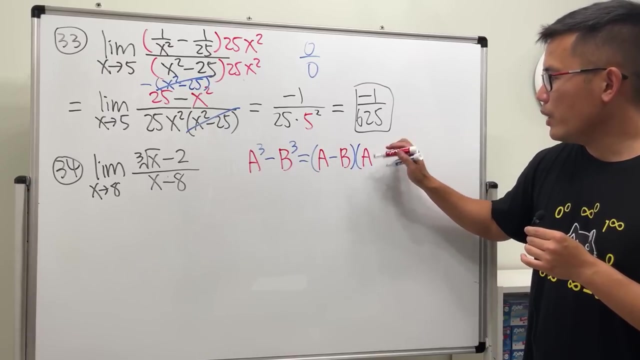 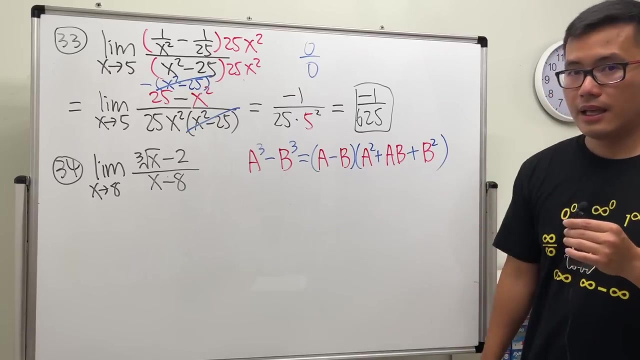 as the difference of two cubes. I will show you, guys that, on the side, When we have a to the third power minus b to the third power, this right here is equal to a minus b times a squared plus a, b, and then plus b squared. 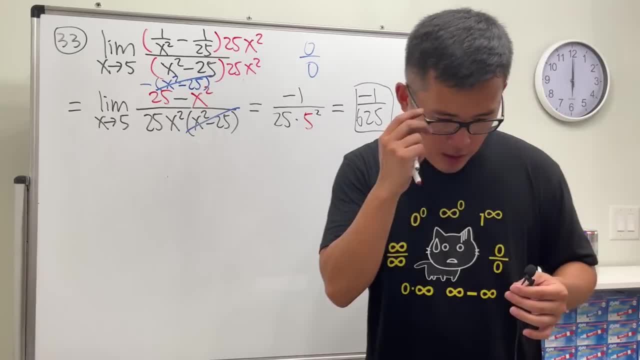 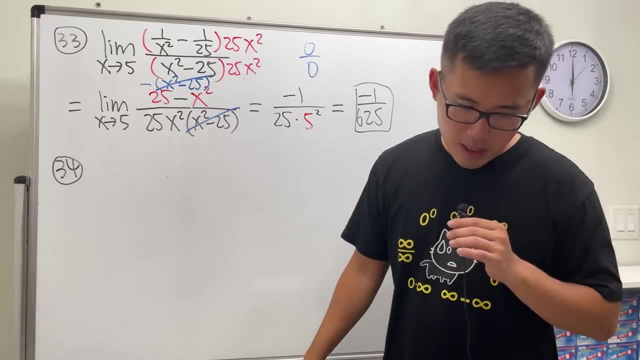 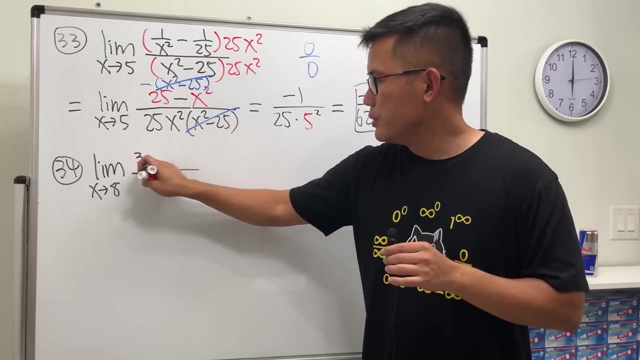 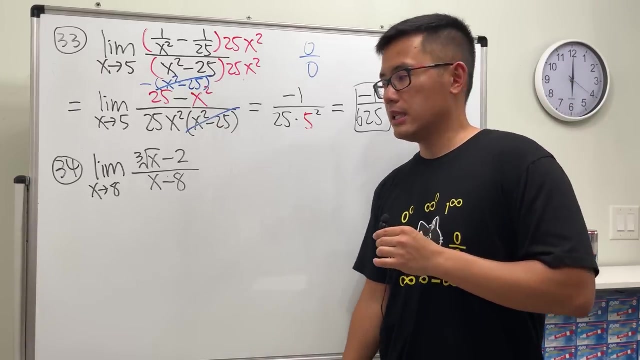 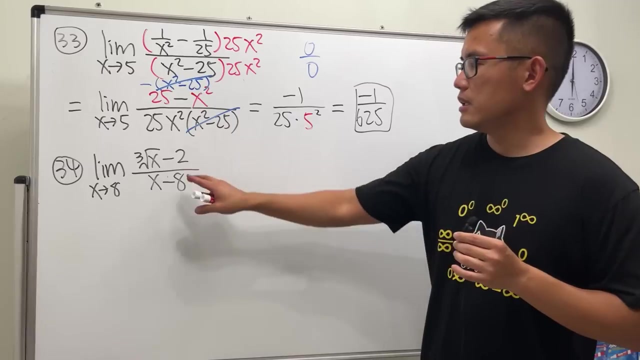 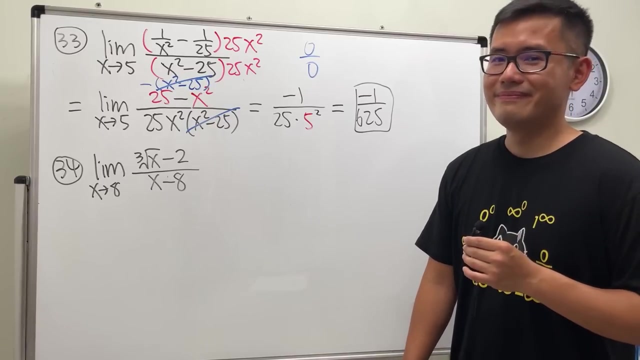 alright, ladies and gentlemen. number 34 limit as X approaching 8, and then we have the cube root of x minus 2 over x minus 8. how do we do this? we can multiply by the country the conjugate to kind of heat to get rid of the cube root. That's possible. But let's look at the following. 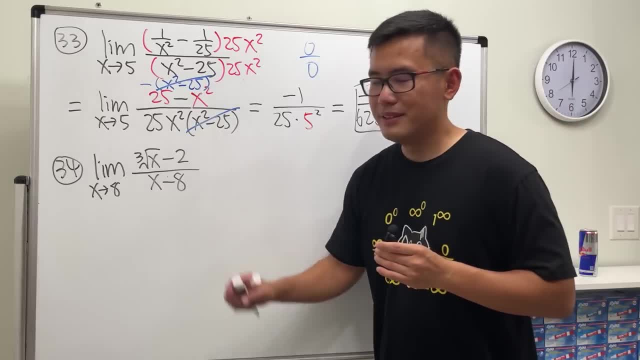 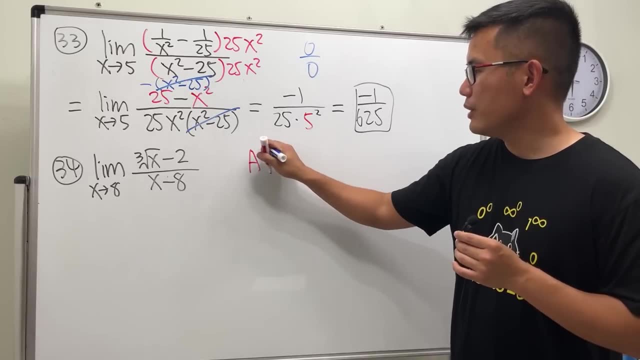 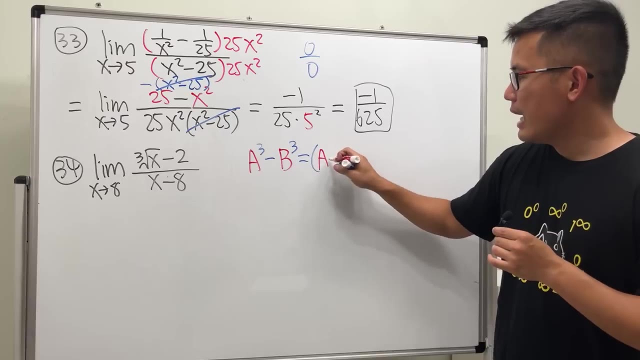 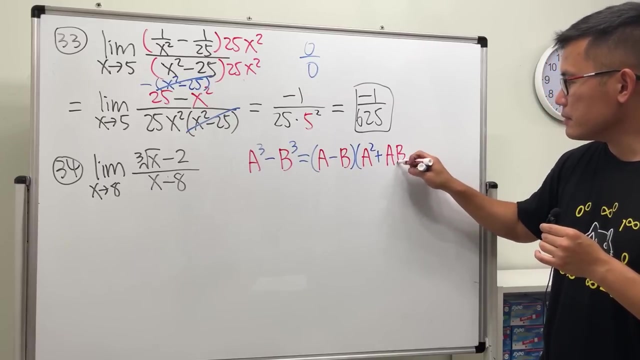 all right. Firstly, we can factor this as the difference of two cubes. I will show you guys that, on the side, When we have a to the third power minus b to the third power, this right here is equal to a minus b times a square plus ab, and then plus b square. What's? 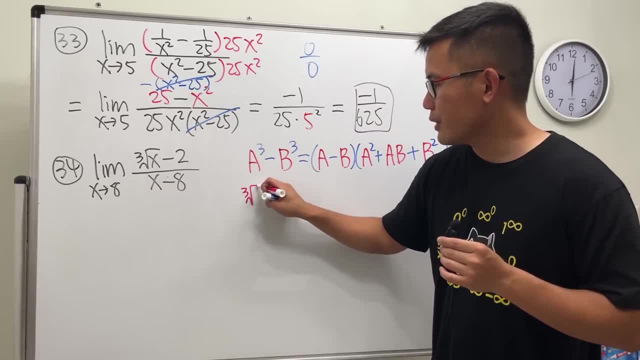 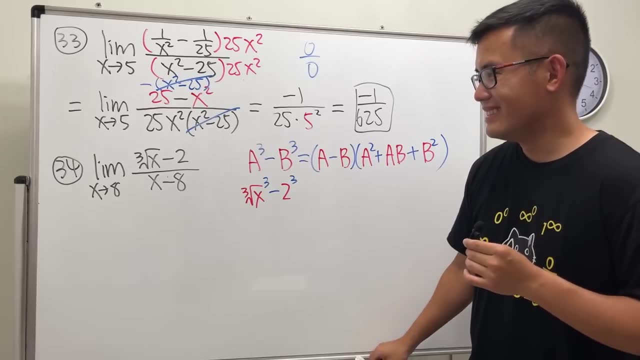 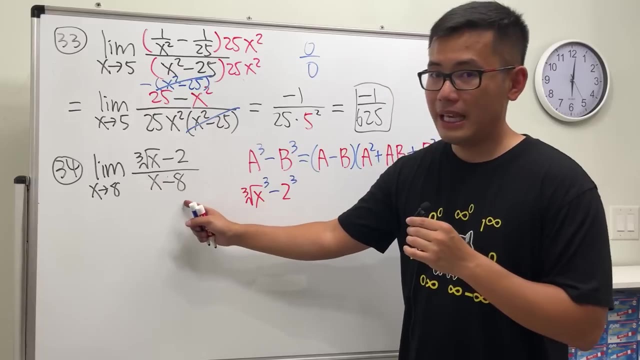 x. x is the same as the cube root of x to the third power. What's 8?? It's the same as 2 to the third power. So I'm just going to put down the factor right here. I don't want to write this down, just put it here. So x minus 8, apply the formula. 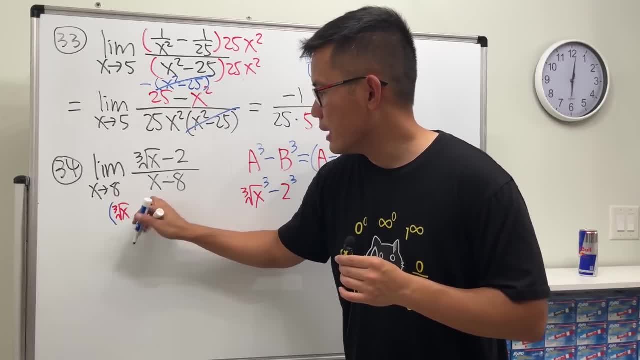 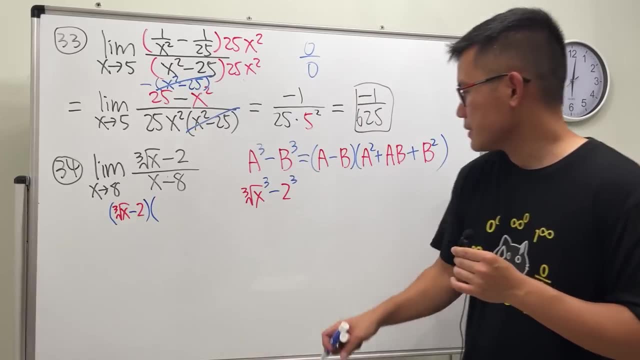 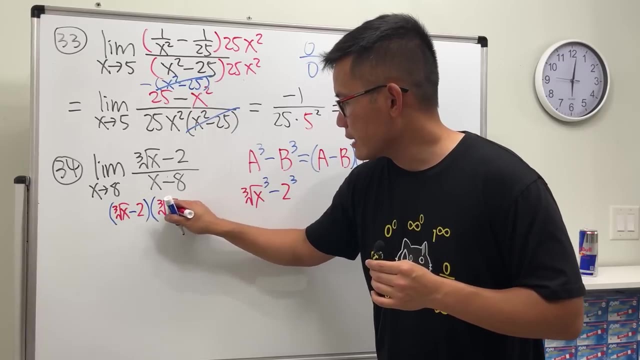 we will first get cube root of x minus 2.. You see, they cancel already, huh, And we just have to figure out the rest, which is okay, we have to square this. So I'm going to just put it down like this: The cube root of x, yeah, And then we have to square it. 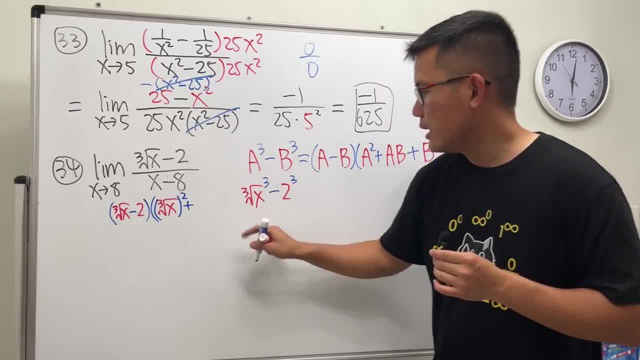 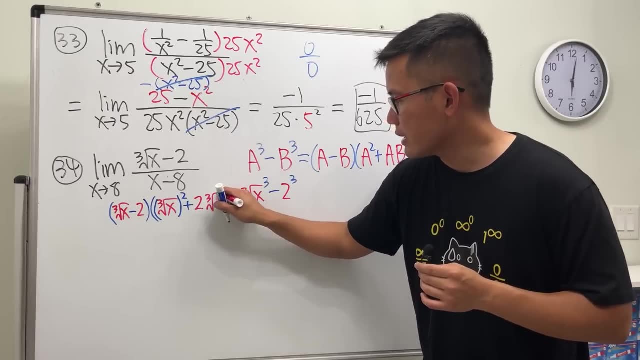 and then plus a, b, so we have to multiply these two together, So that's 2, and that, so it's 2, and the cube root of x. And lastly, we have to put b squared, which is 2 squared, which is just. 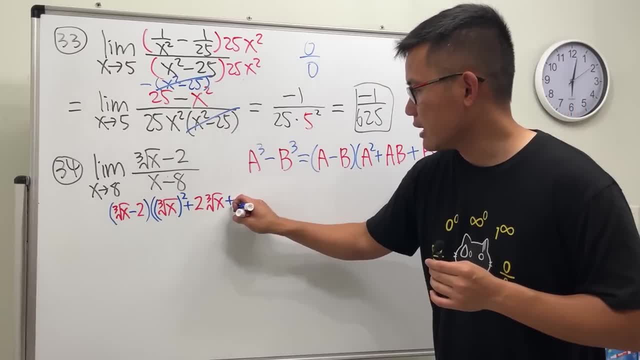 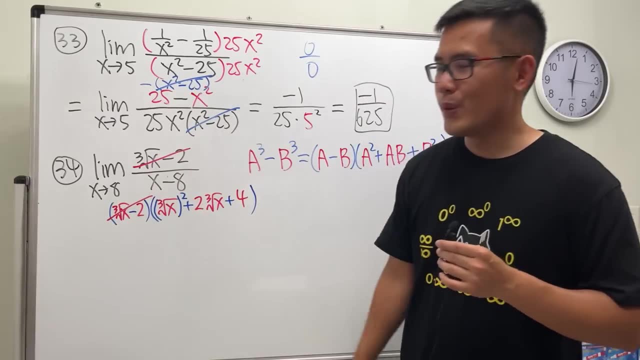 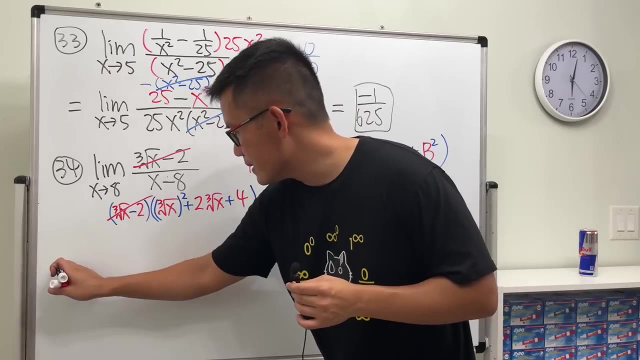 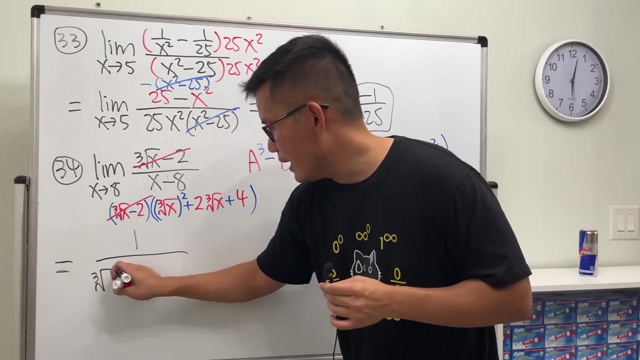 a plus 4.. So right here we have the plus 4.. Very nice, huh, Cancel, cancel. All right, Now let's put the 8 into here here, And we have 1 on the top over here, cube root of 8.. And then we square that and then plus. 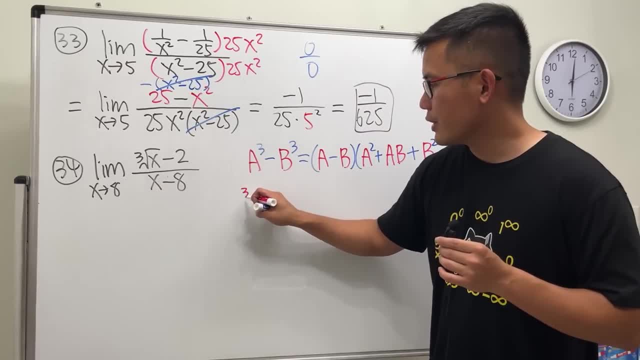 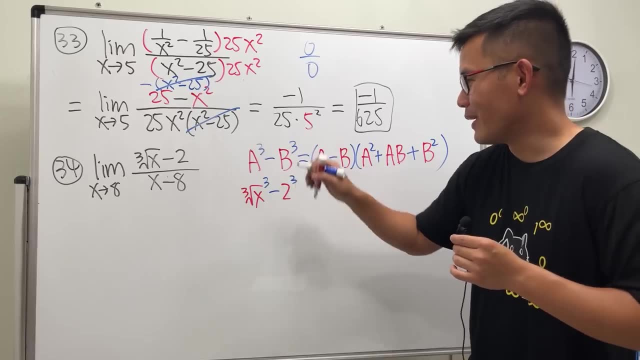 What's x? x is the same as the cube root of x to the third power. What's 8?? It's the same as 2 squared. I mean 2 to the third power. So I'm just going to put down the factor in right here. 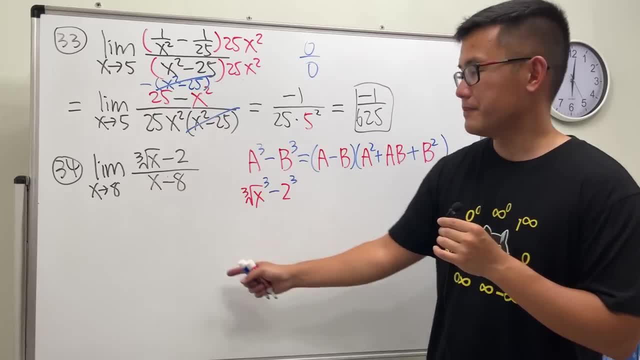 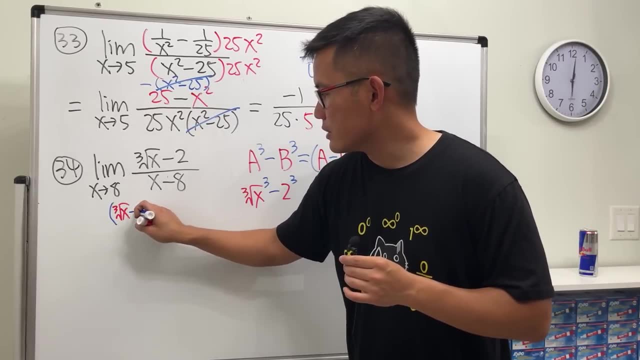 I don't want to write this down, Just put it here. So x minus 8, apply the formula. We will first get cube root of x minus 2.. You see, they can solve already, huh, And we just have to figure out the rest. 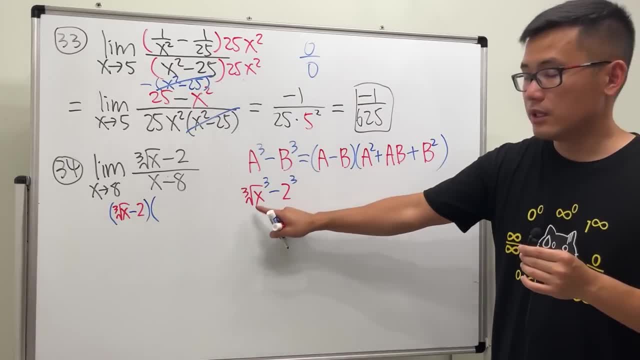 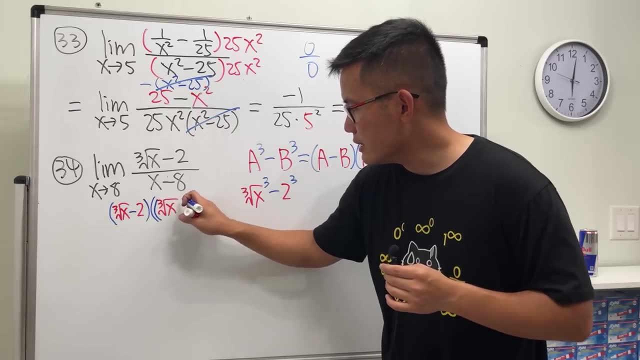 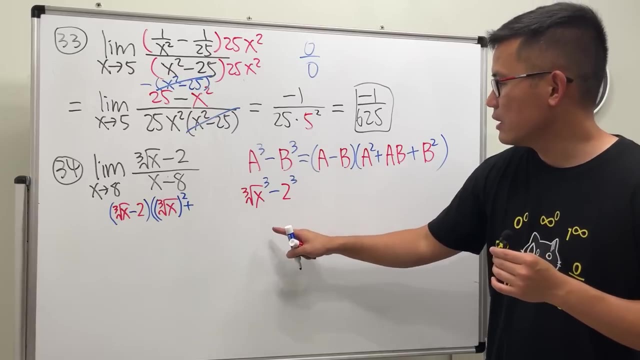 which is okay. we have to square this. So I'm going to just put it down like this: The cube root of x, Yeah, And then we have to square it, And then plus a, b, So we have to multiply these two together. 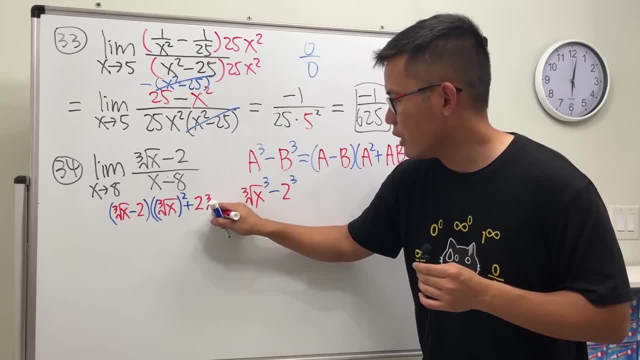 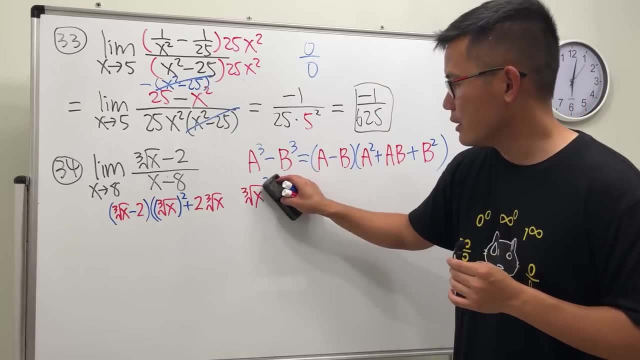 So that's 2 and that, So it's 2 and the cube root of x. And, lastly, we have to put a b squared, which is 2 squared, which is just a plus 4.. So, right here we have the plus 4.. 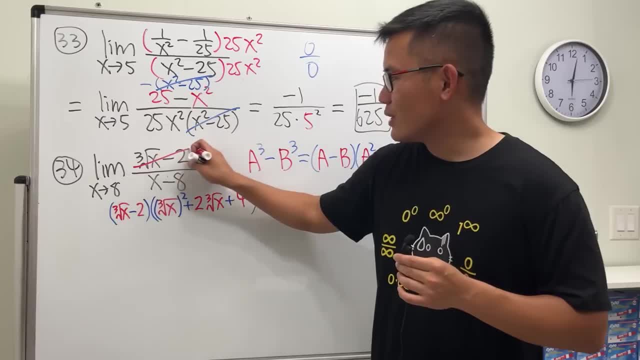 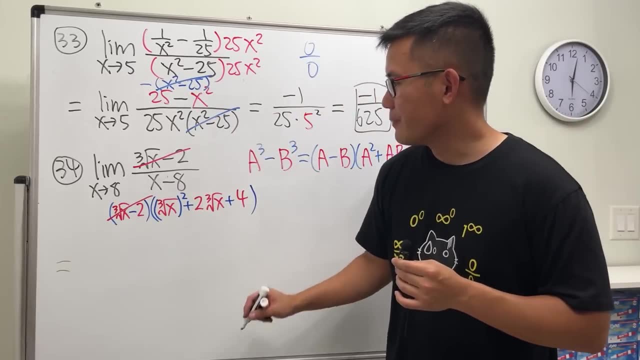 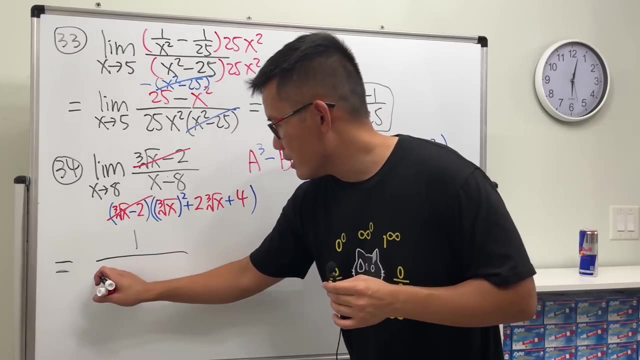 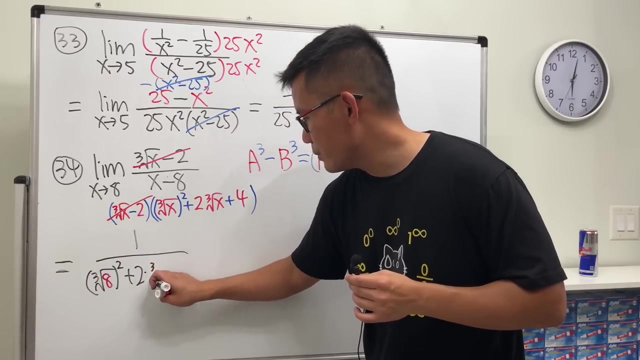 Very nice, huh, Cancel, Cancel, Wow, All right, Now let's put the 8 into here here And we have 1 on the top Over here, Cube root of 8.. And then we square that And then plus 2 times the cube root of 8.. 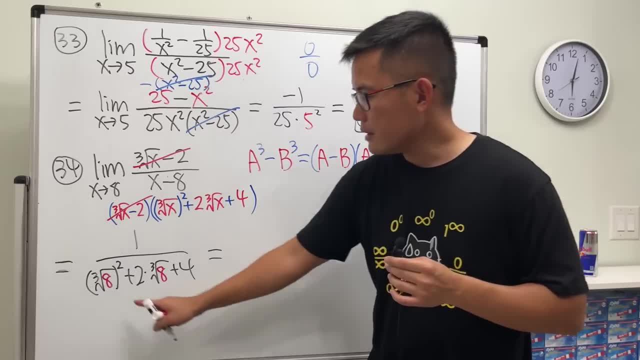 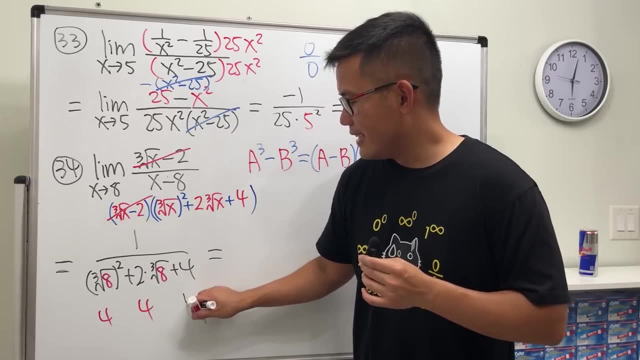 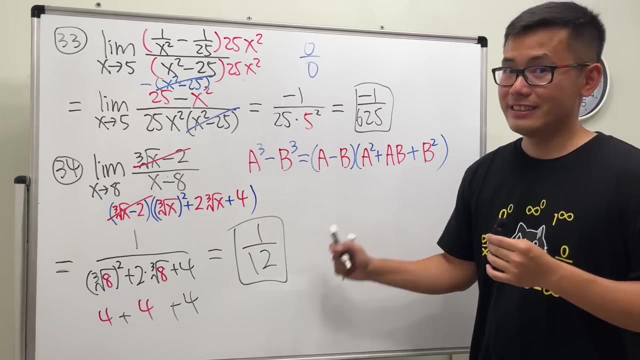 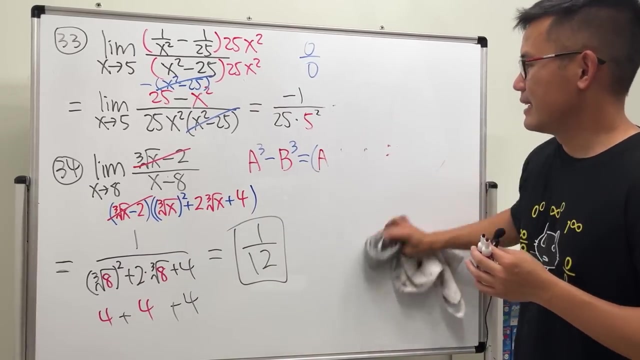 And then we add the 4. This is 2 inside Square that we get 4. This is 2 times 2 is 4. 12. 1 over 12. Done Ladies and gentlemen, that is number 34.. 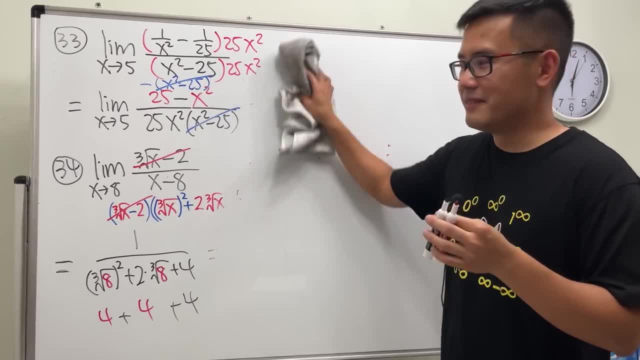 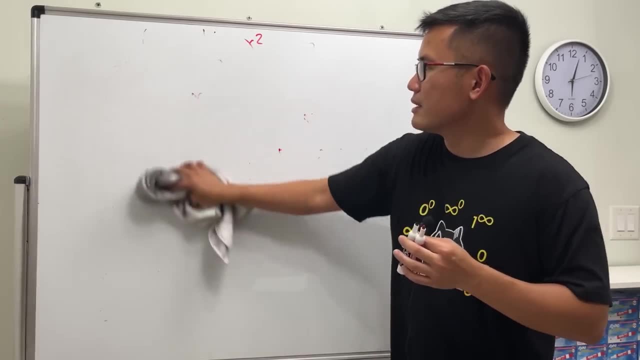 All right, I'm going to do one more question with this marker And I'm going to change to a better marker So that way you guys can see this better. I have a brand new marker over here And then later on. 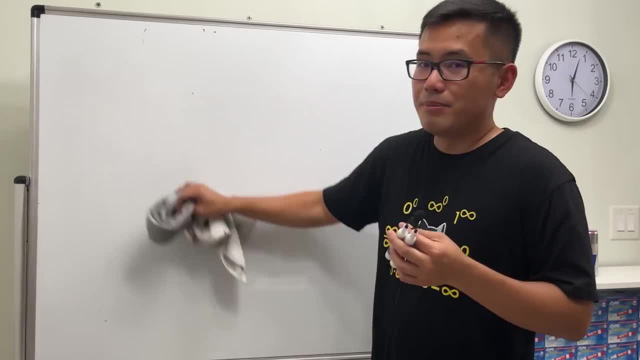 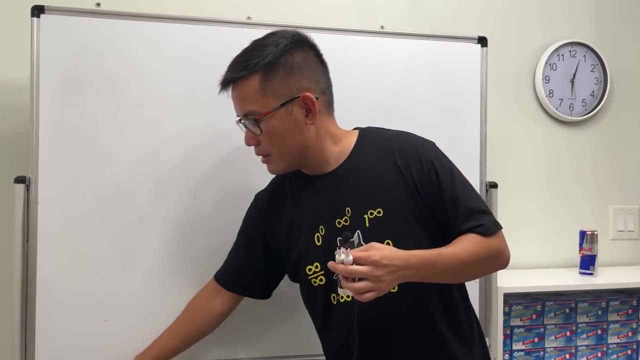 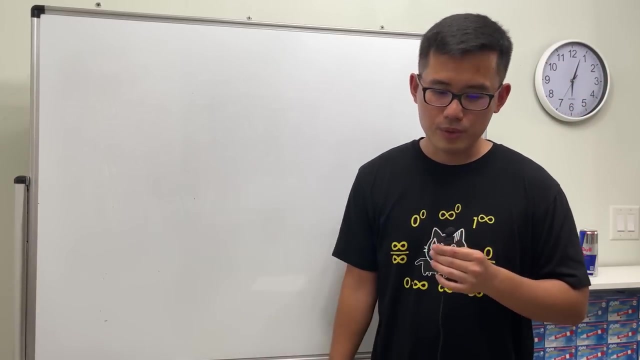 when I do the smaller questions And sometimes if you just let the marker sit, you know it's going to come back alive. If you just put a marker like this for a while then yeah, it will come back alive And you can solve like 2 or 3 integrals. 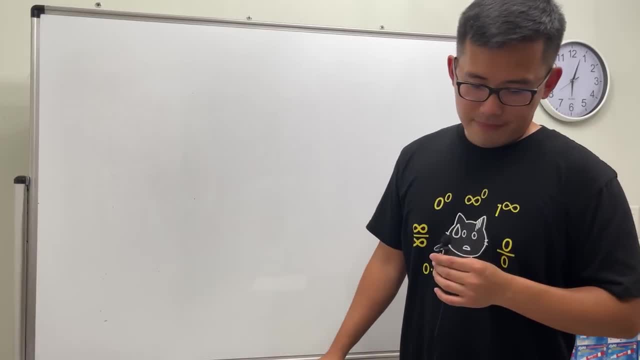 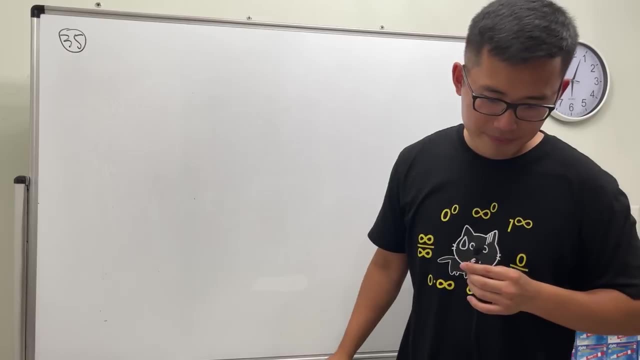 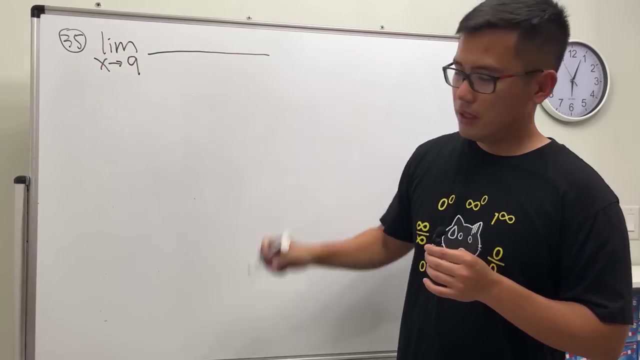 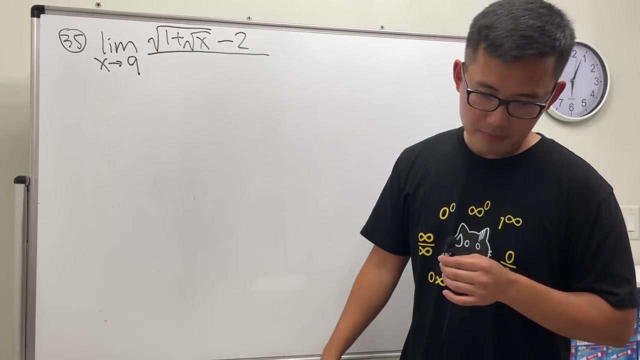 before it tries out again, But anyway, number 35.. This is called nested square root, Because you have a square root inside of a square root, Limit x approaching 9.. And we have square root 1 plus square root of x and then minus 2. 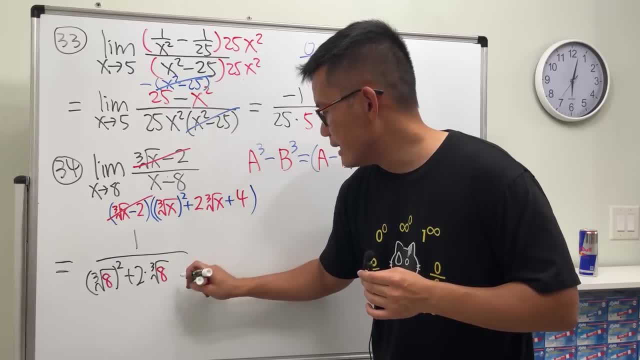 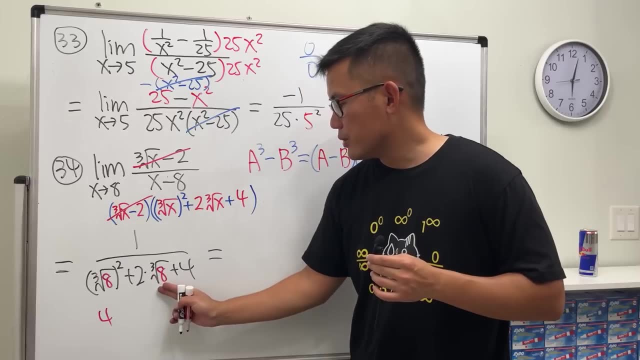 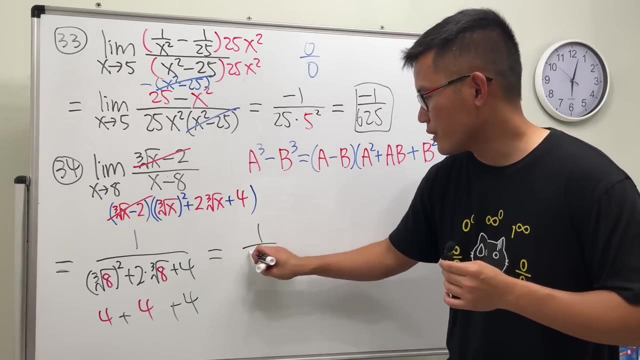 2 times the cube root of 8, and then we add the 4. This is 2 inside square that we get 4.. This is 2 times 2 is 4.. 12. 1 over 2.. 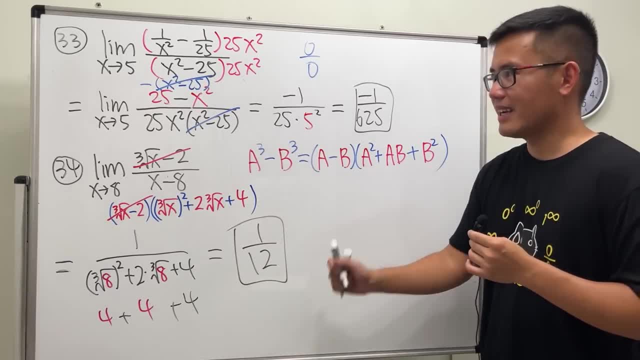 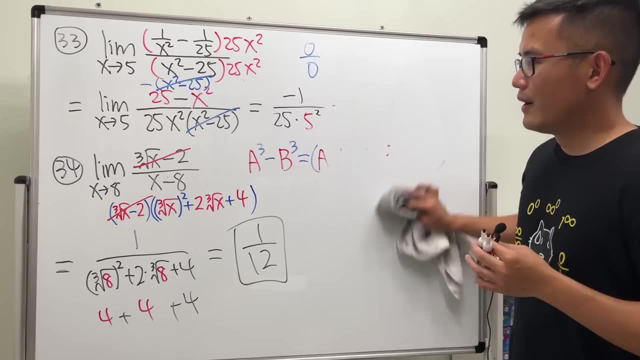 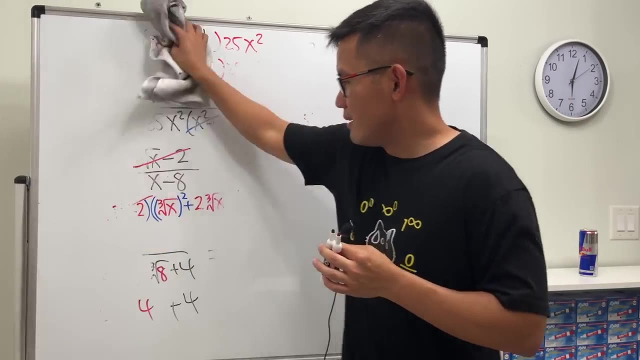 12. Done, Ladies and gentlemen, that is number 34.. All right, I'm going to do one more question with this marker and I'm going to change to a better marker, so that way you guys can see like you guys can see this better. 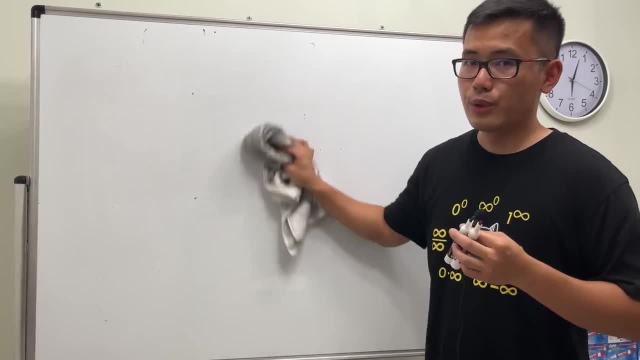 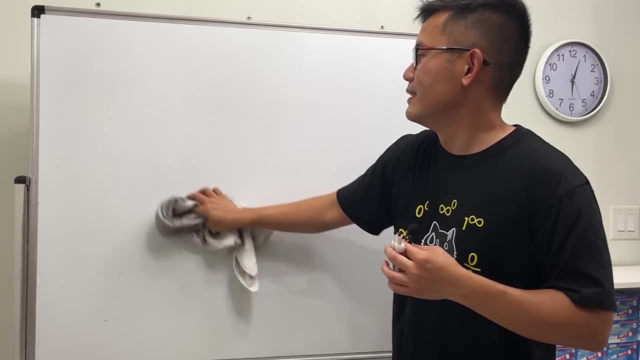 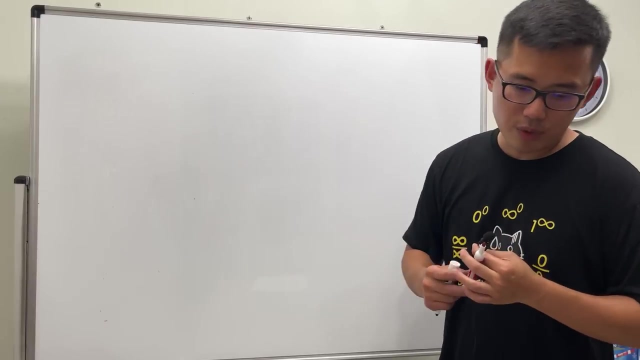 I have a brand new marker over here, and then later on when I do the smaller questions, and sometimes if you just let the marker sit, you know it's going to come back alive. if you let me, if you just put a marker like this for a while, then, yeah, it will come back. 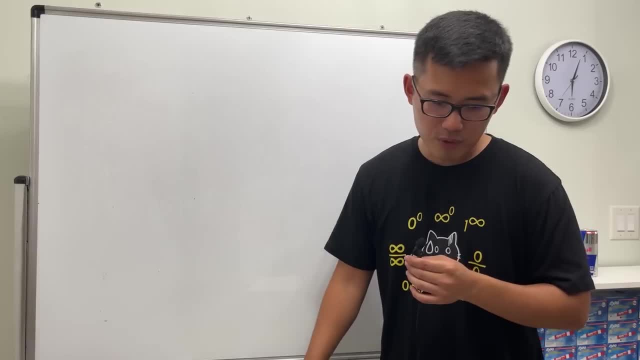 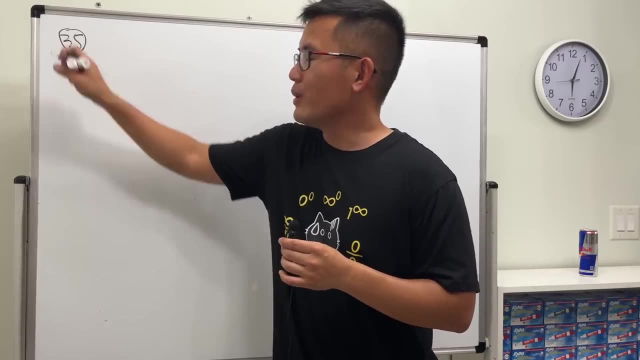 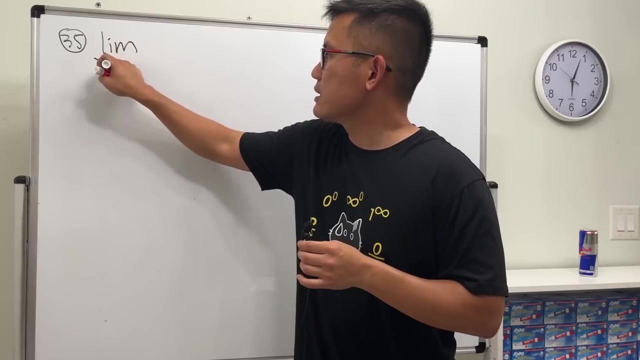 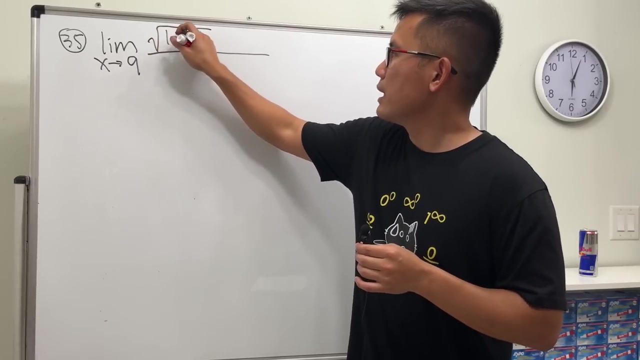 alive and you can solve like two or three integrals before it dries out again. but anyway, number 35: this is called nested square root because you have a square root instead of a square root, limit x approaching 9 and we have square root 1 plus square root of x. 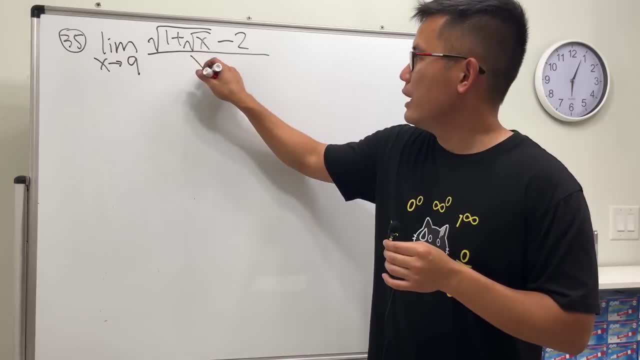 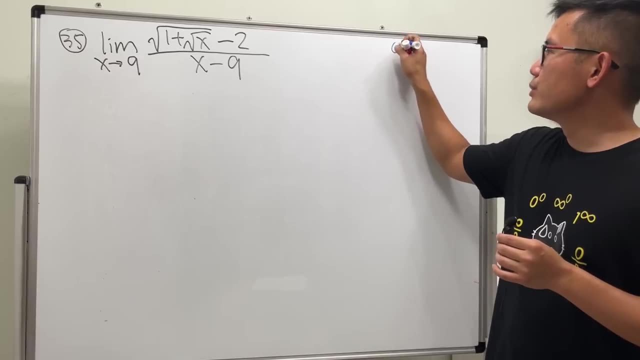 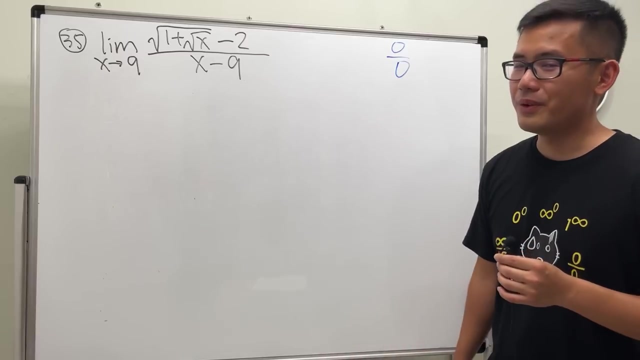 and then minus 2 over x, minus 9. here's the deal. plugging 9 into all the x's, yes, you get 0 over 0. i don't remember if i checked earlier. yeah, it was obvious, it was 0 over 0 for number 34. all right, for number 35. here let's go ahead and multiply by a conjugate first to get. 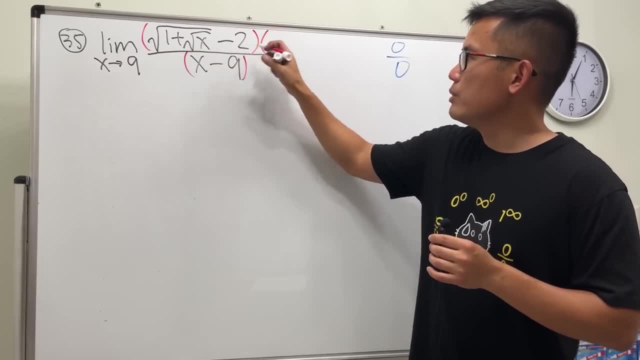 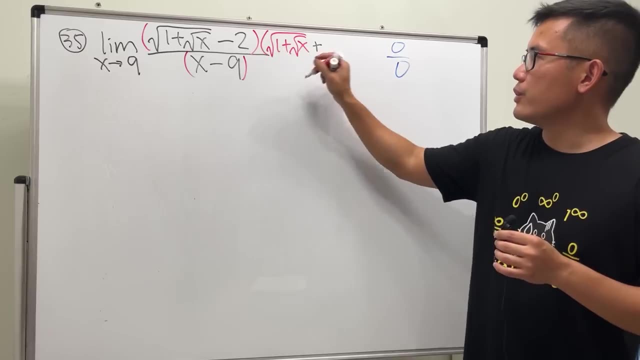 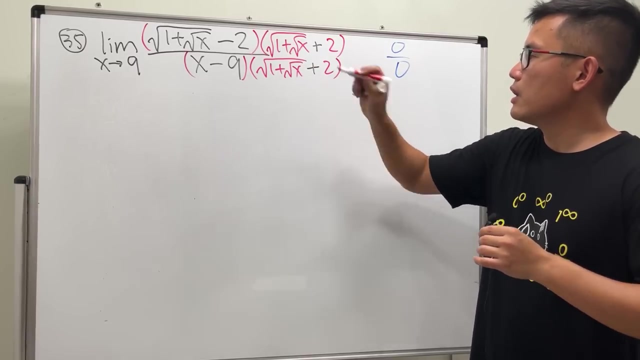 rid of this square root. so i'm going to multiply the top and bottom by square root of 1 plus the square root of x, and change this minus to a plus, and then the two stays, and then let's do the same on the bottom. cool, now this right here is the limit as x approaching 9. 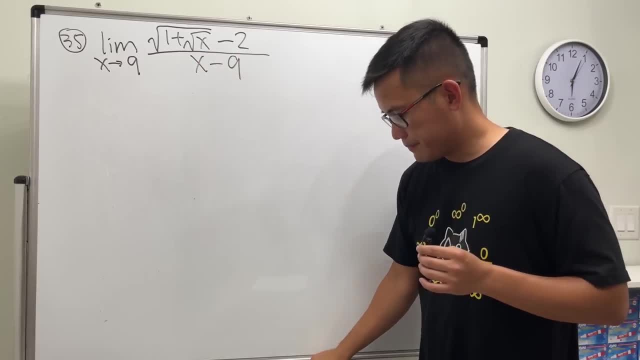 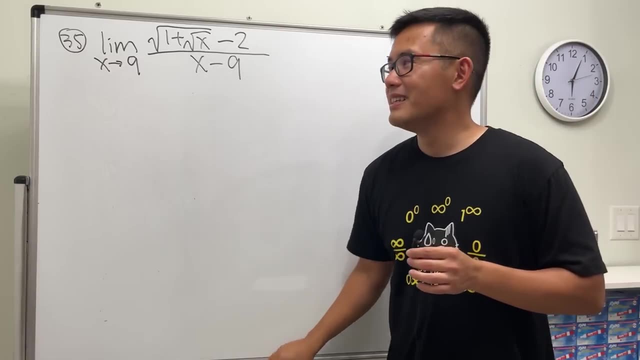 over x minus 9.. Here's the deal: Plugging 9 into all the x's, yes, you get 0 over 0. I don't remember. if I checked that earlier, Yeah, it was 0 over 0 for number 34.. 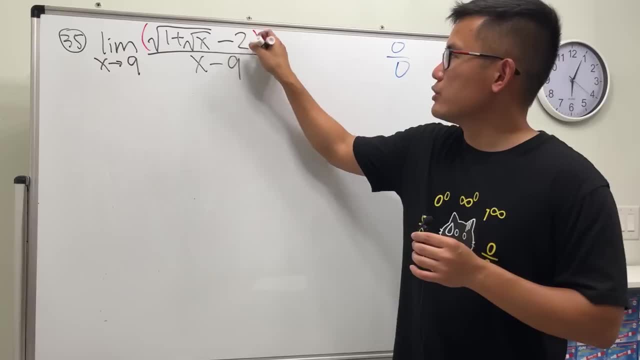 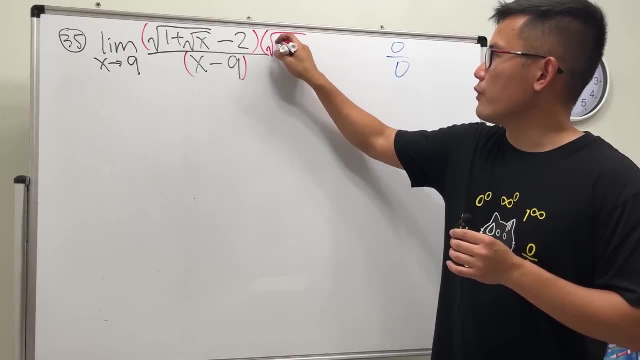 All right For number 35. here let's go ahead and multiply by a conjugate, first to get rid of this square root. So I'm going to multiply the top and bottom by square root of 1 plus the square root of x and change this minus to a plus. 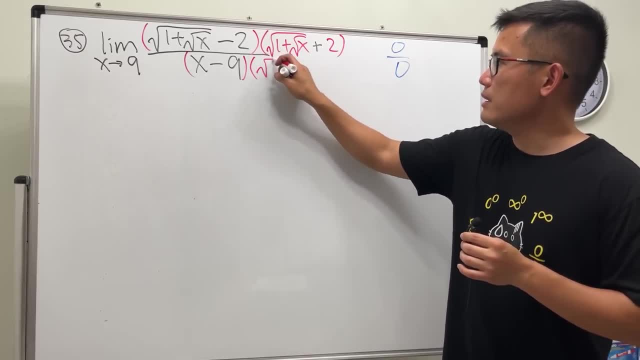 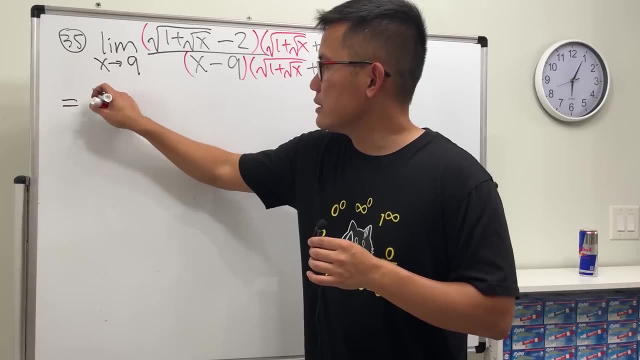 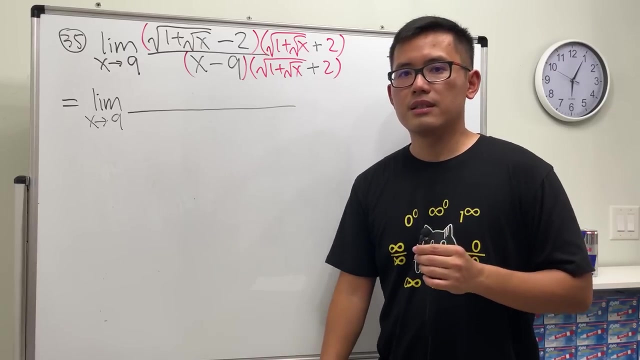 and then the 2 stays. And then let's do the same on the bottom. Cool, Now this right here is the limit as x approaching 9.. How do we multiply all the conjugate? Just square the first thing, so that the big square root will cancel. 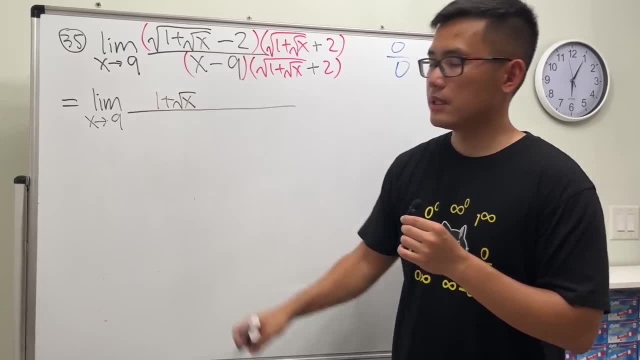 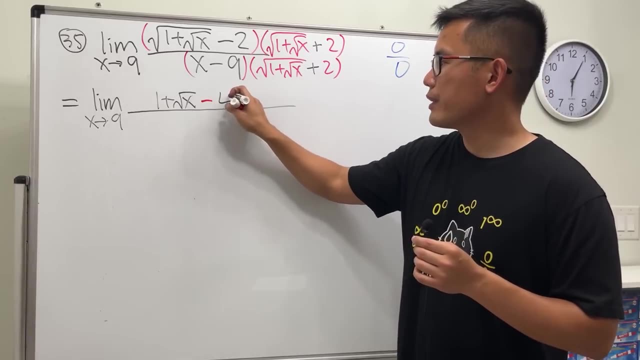 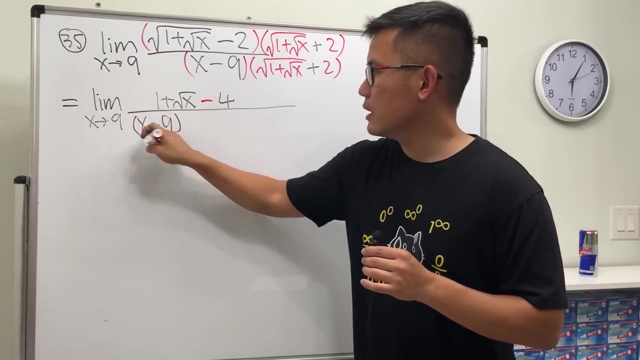 So we have 1 plus square root of x. What's next? Minus 2 square, that, which is 4.. Good, On the bottom, don't do anything, Just write it down. So we have x minus 9, and then. 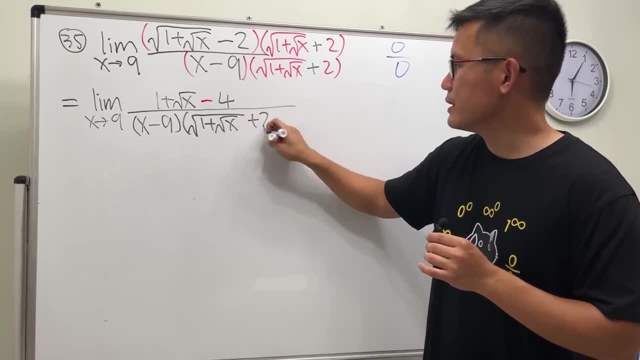 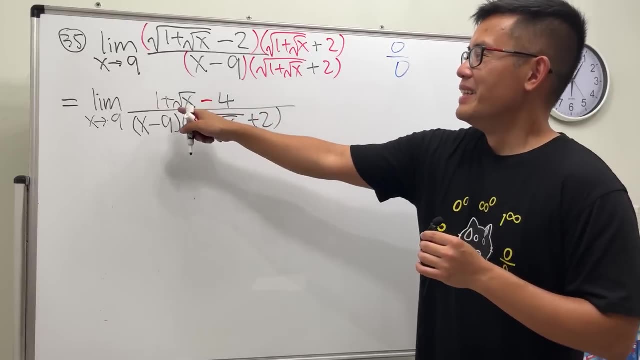 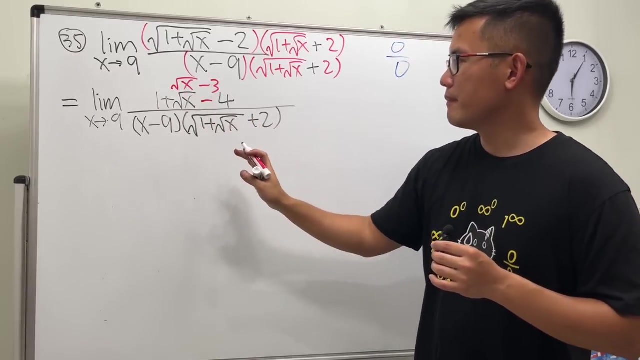 square root of 1 plus square root of x and then plus 2.. Good, On the top we can actually just do 1 minus 4, which is square root of square root of x, or 1 minus. it's just this square root of x minus 3.. 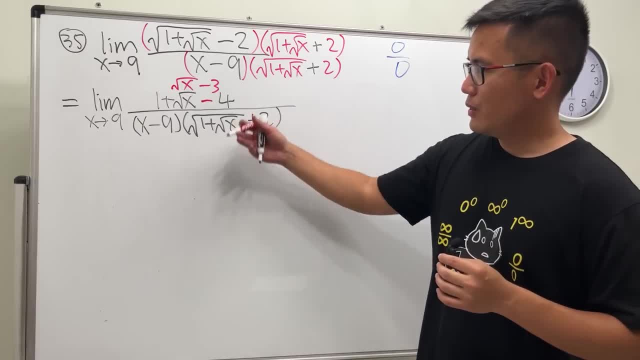 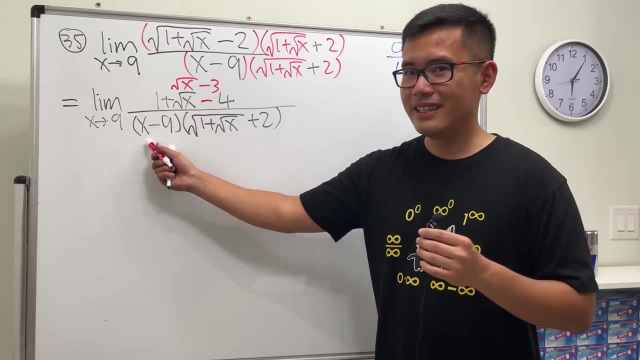 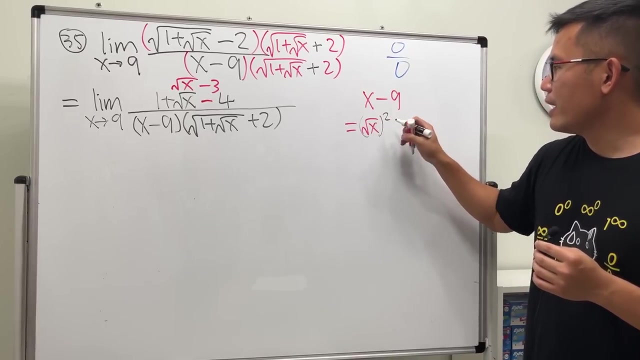 Yeah, What do we do next? Do you want to multiply the conjugate again? Sure, Be my guest, But you know it. This guy, x minus 9 is the same as square root of x square minus 3 square, isn't it? 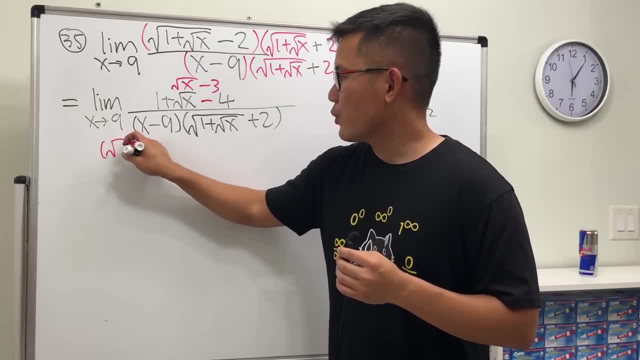 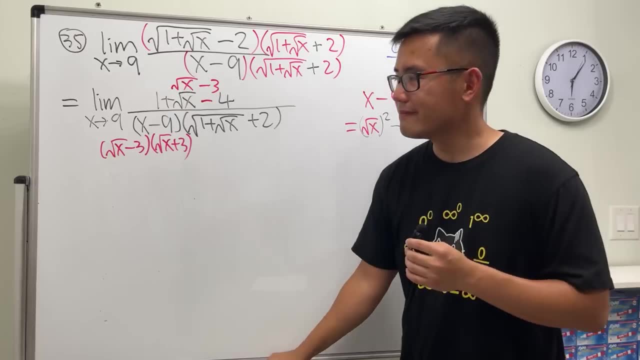 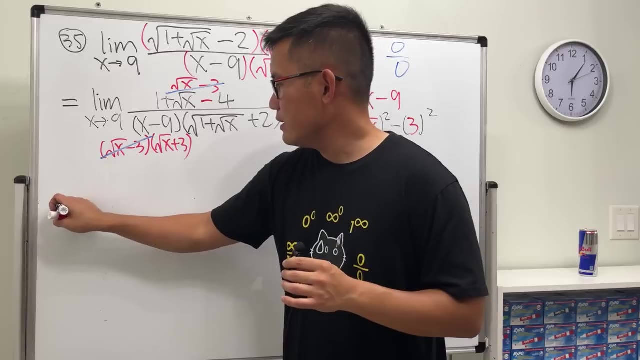 So we can factor this as square root of x minus 3 times square root of x plus 3.. Cancel the top with that. No more 0 over 0.. Yay, Finally, 1 over. don't forget this. We have a square root of. 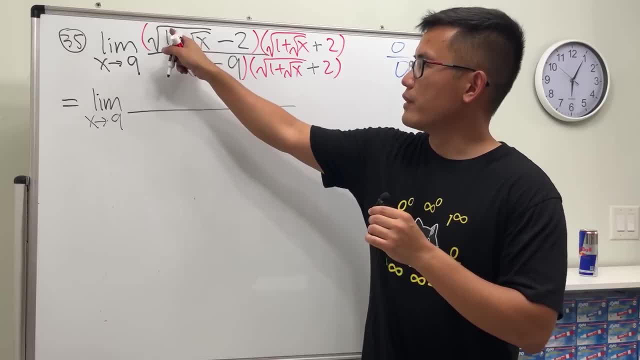 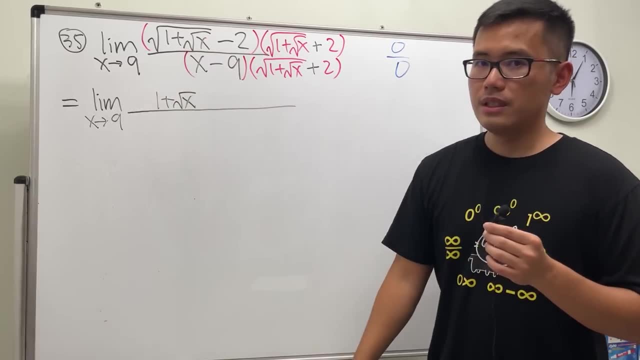 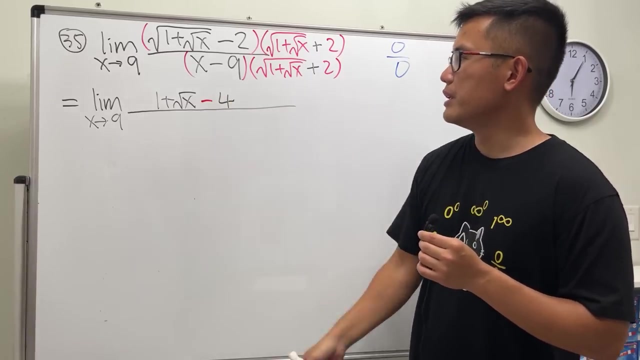 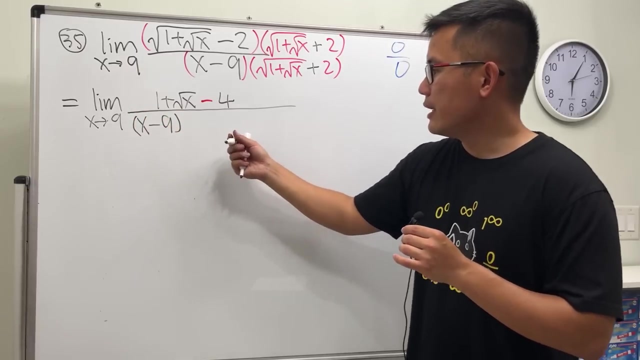 how do we multiply all the conjugate? just square the first thing so that the big square root will cancel. so we have 1 plus square root of x. what's next? minus 2, square, that which is 4. good, on the bottom, don't do anything, just write it down. so we have x minus 9, and then 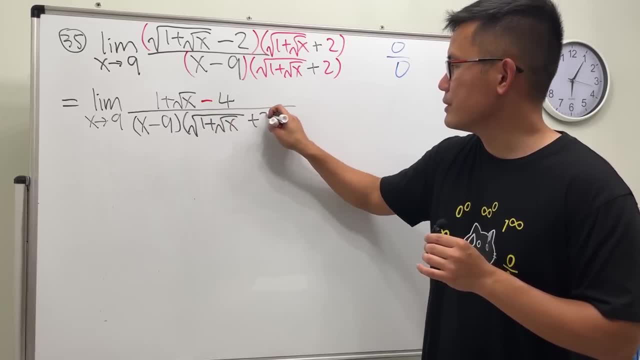 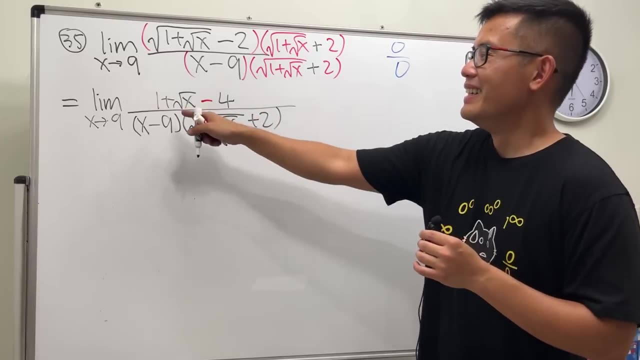 square root of 1 plus square root of x and then plus 2. good, on the top we can actually just do 1 minus 4, which is square root of square root of x, or 1 minus. it's just this square root of x minus 3. 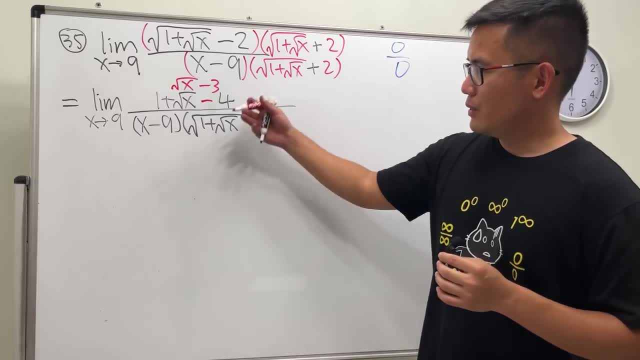 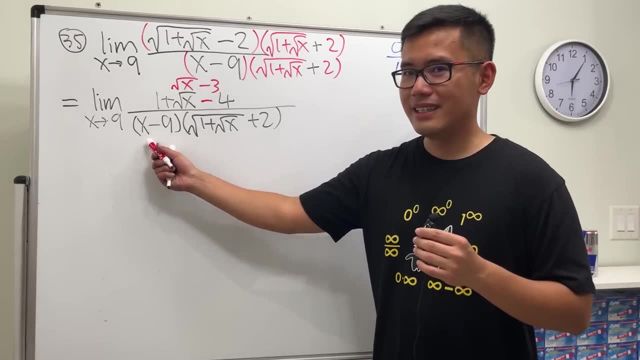 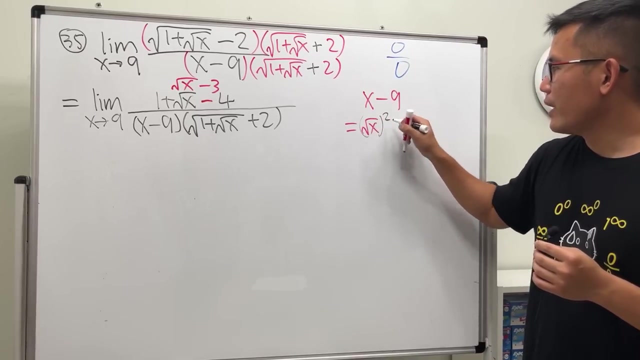 yeah, what do we do next? do you want to multiply the conjugate again? sure, be my guest, but you know it. this guy, x minus 9 is the same as square root of x square minus 3 square, isn't it? so we can factor this as: 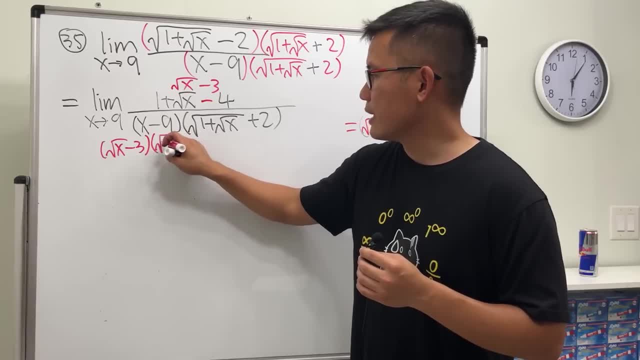 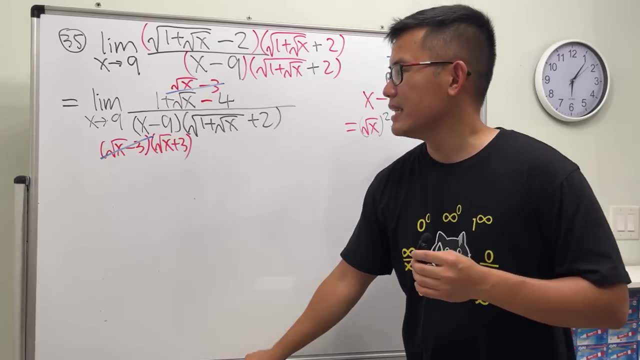 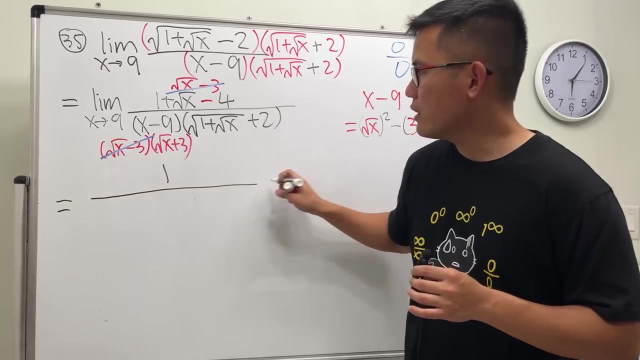 square root of x minus 3 times square root of x plus 3. cancel the top with that. no more 0 for 0. okay, finally, 1 over. don't forget this: we have a square root of x is 9, just plug in and then plus 3. 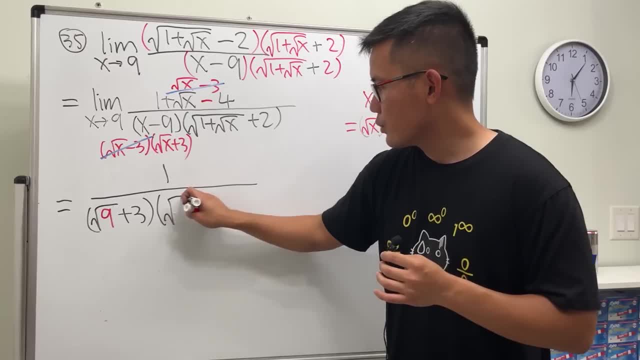 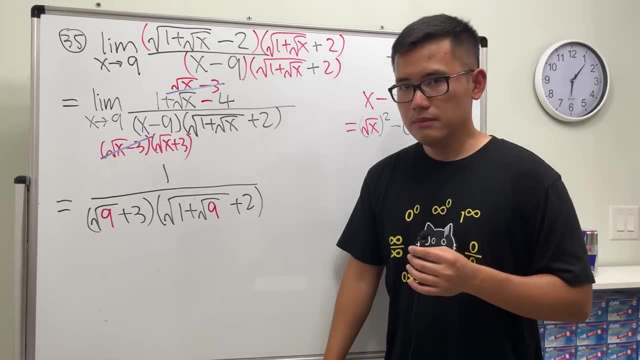 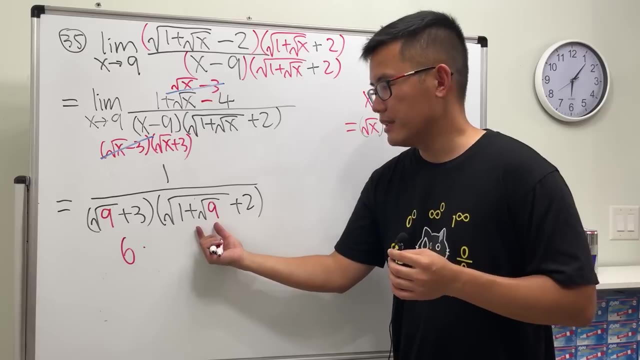 so this is the first factor, and then square root 1 plus square root of 9, and then plus 2- just work this out- is 3, plus 3 is 6, times this is 3, plus 1 is 4, square root of 4 is 2, 2 plus 2 is. 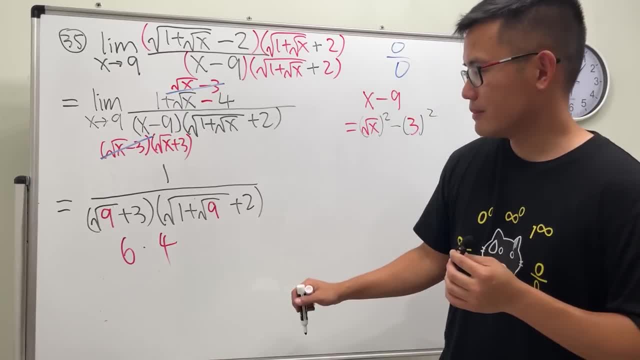 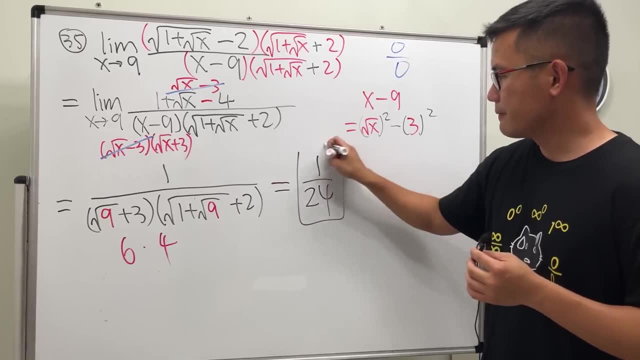 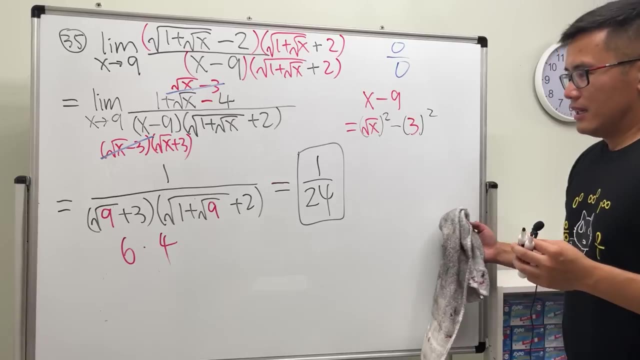 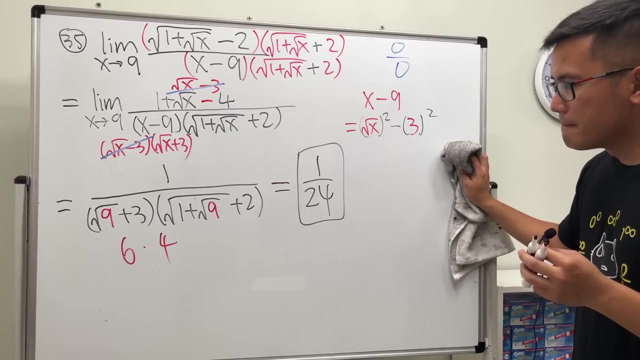 4, so we have 1 times 4,. well, we have 6 times 4, and 1 over 24,. yes, I did it right. I believe so, yeah. yeah, by the way, that is number 35, when we have double square roots, you. 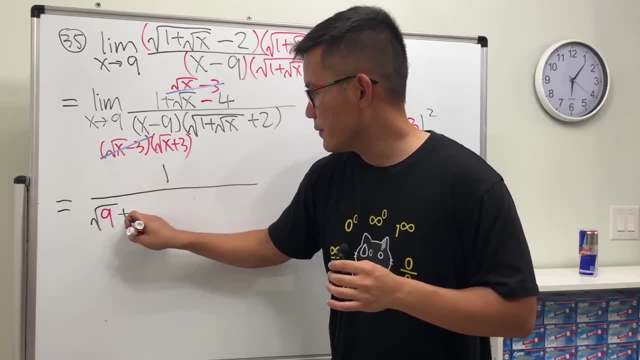 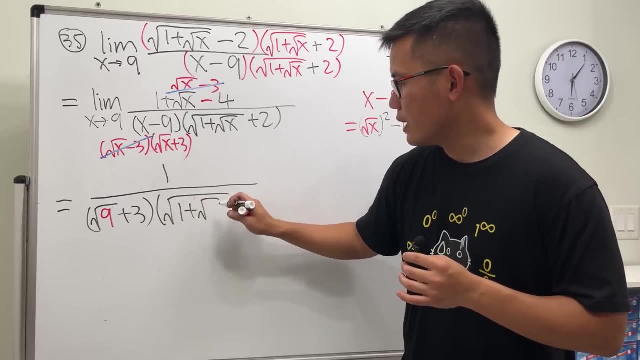 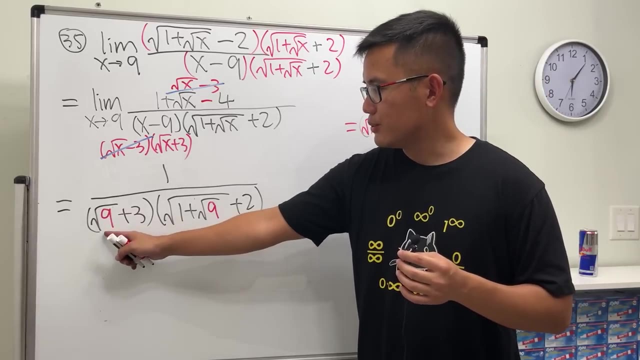 x is 9.. Just plug in And then plus 3.. So this is the first factor, And then square root 1 plus square root of 9 and then plus 2.. Just work this out. This is 3 plus 3 is 6. 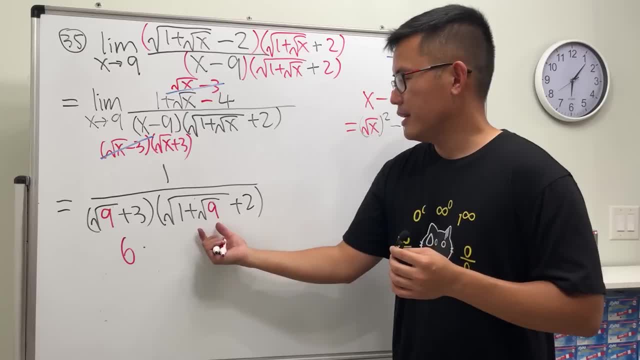 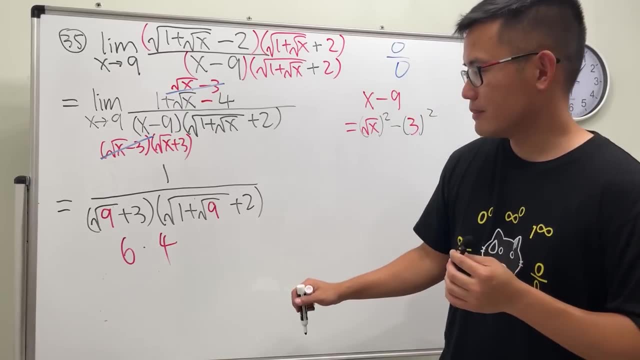 times this is 3 plus 1 is 4.. Square root of 4 is 2.. 2 plus 2 is 4.. So we have 1 times 4.. We have 6 times 4.. So we have 6 times 4.. 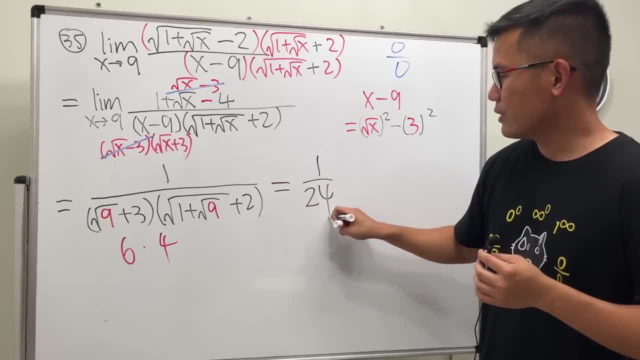 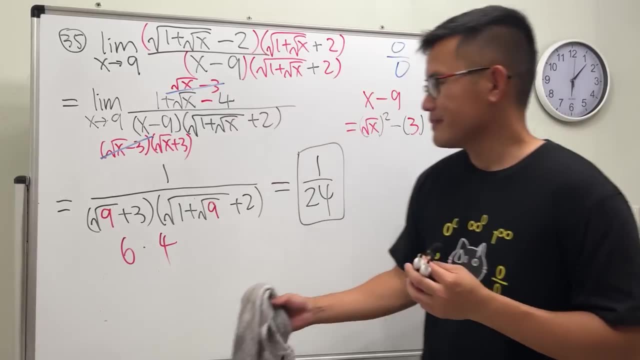 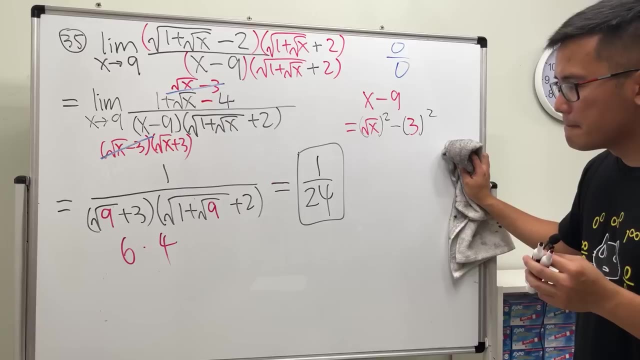 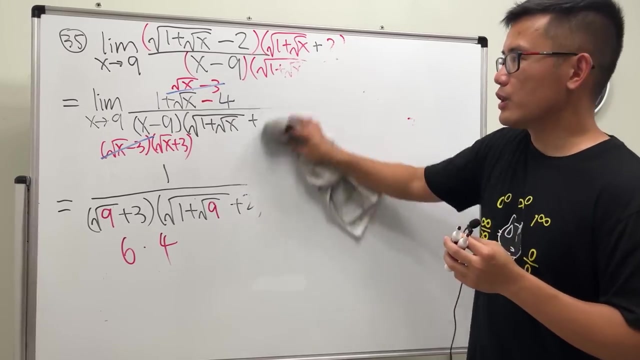 And 1 over 24.. Yes, I did it right. I believe so, Yeah, yeah, By the way, that is number 35.. When we have double square roots, you can do the conjugate twice or just take advantage of that. 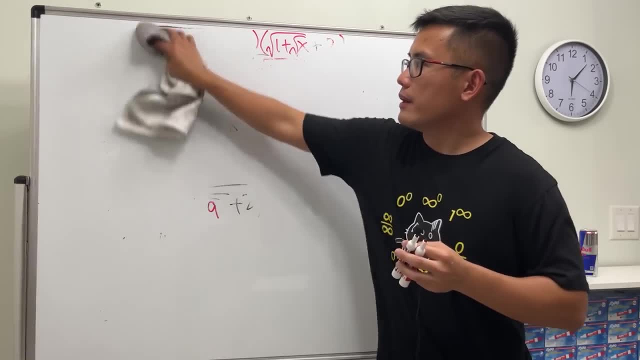 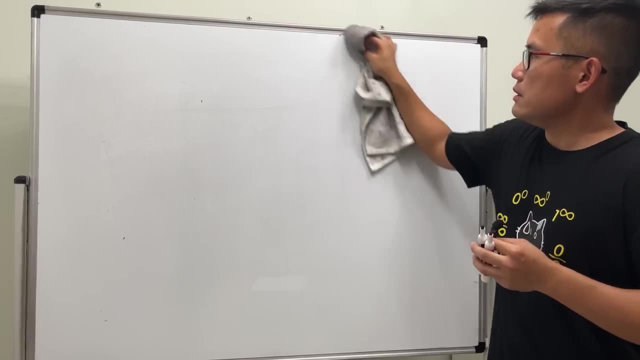 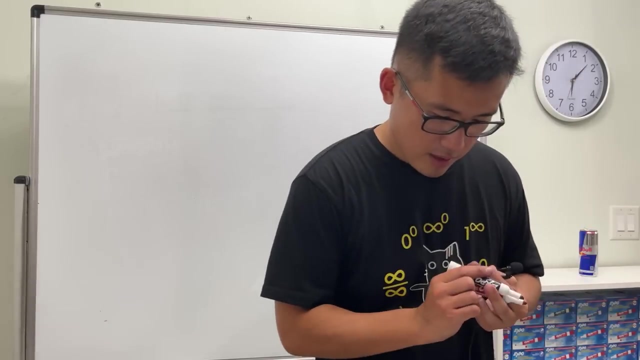 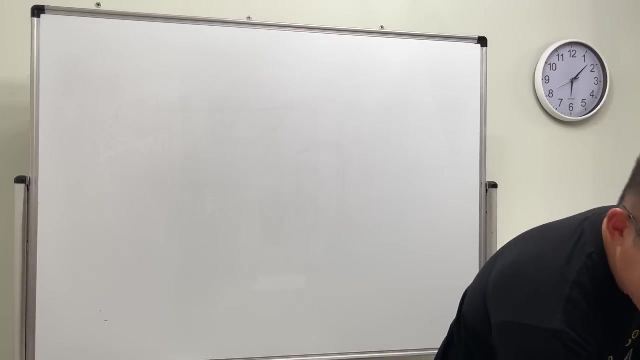 like how we can factor it, like the ways I show you guys Use radicals and a difference of 2 squares or maybe the difference of 2 cubes. Page 4 done. Oh, this sheet of paper is done. Moving on to page 5.. 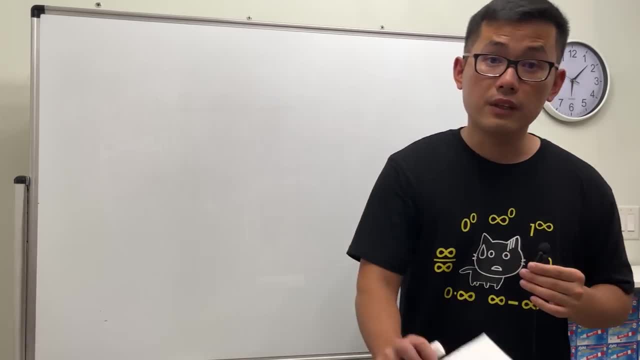 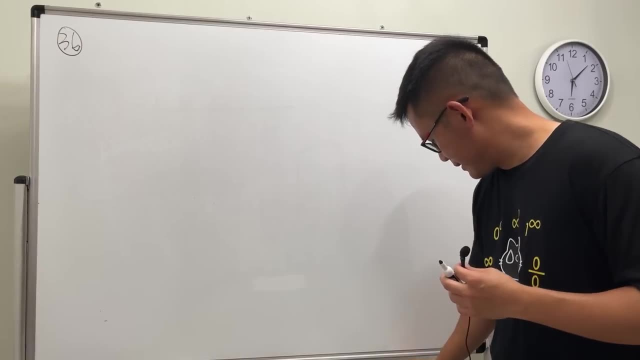 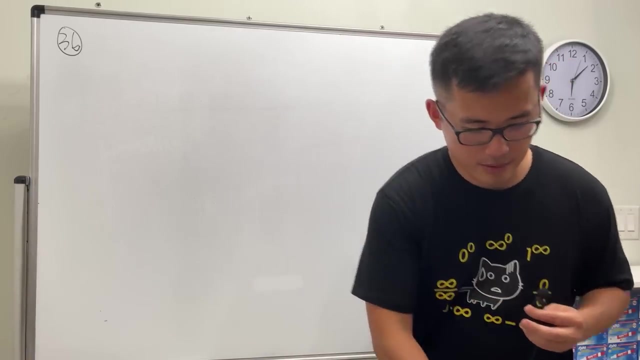 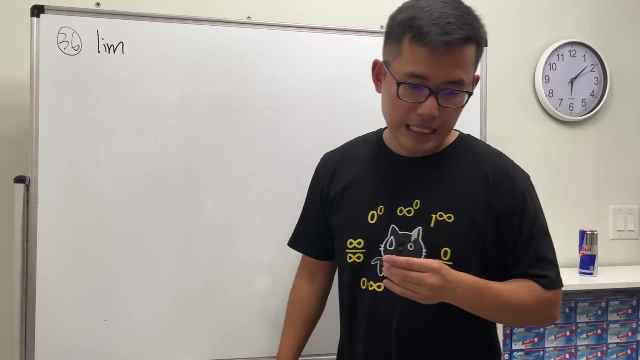 All right, for now we'll be talking about the limit as x approaching infinity. Yeah, yeah, yeah, Look here. All right, number 36.. Here we have the limit, and then we have x approaching infinity, and then we have x approaching infinity. 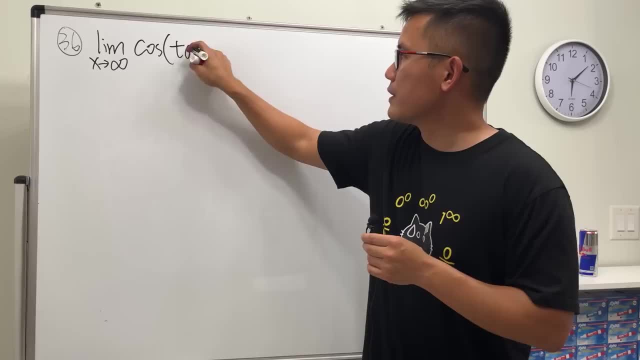 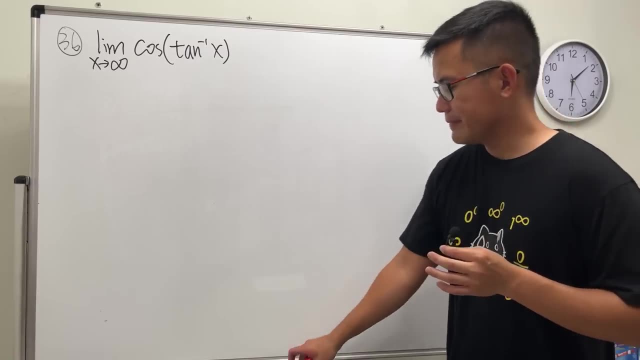 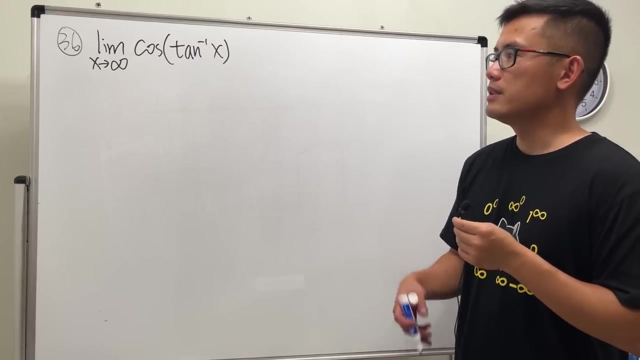 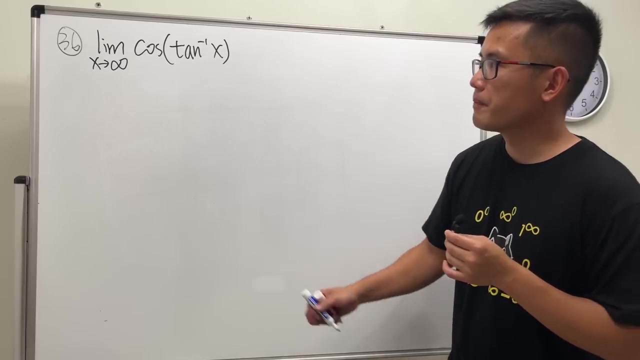 and then we have cosine of inverse tangent of X. okay, so for this kind of questions it really depends on your teacher, your professor, your TA to see how they want you to show work. this is how I will love my students for how I will show work. to help students navigate the computation you can just plug. 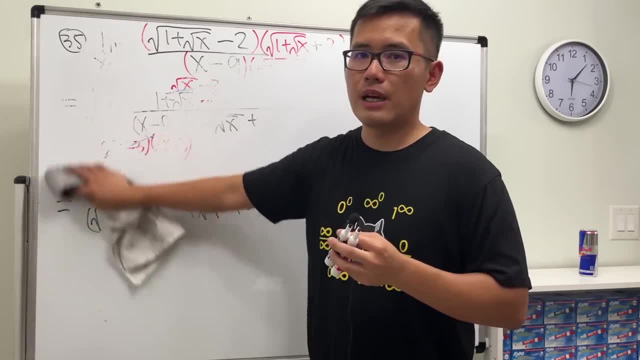 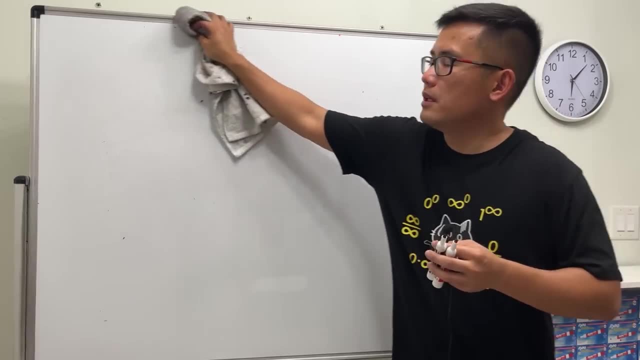 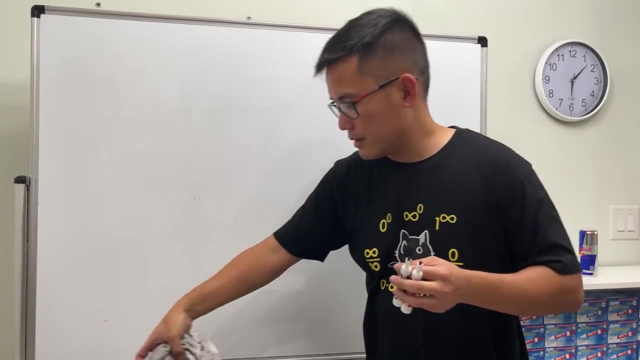 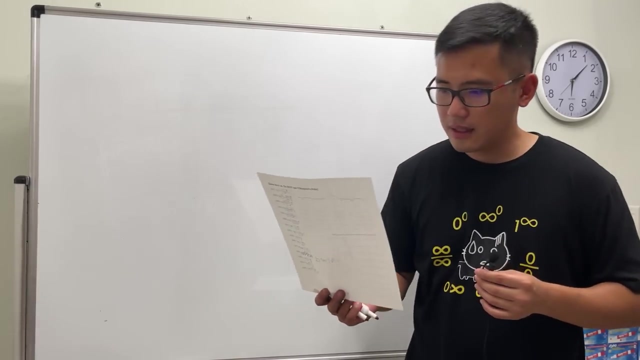 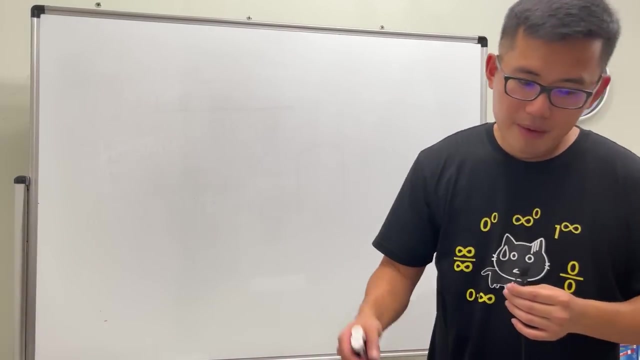 can do the conjugate twice or just take advantage of, like how we can factor it, like the ways I show you guys use radicals and then the difference of 2 squares or maybe the difference of 2 cubes. So page 4, done. oh, this sheet of paper is done. moving on to page 5, alright for. 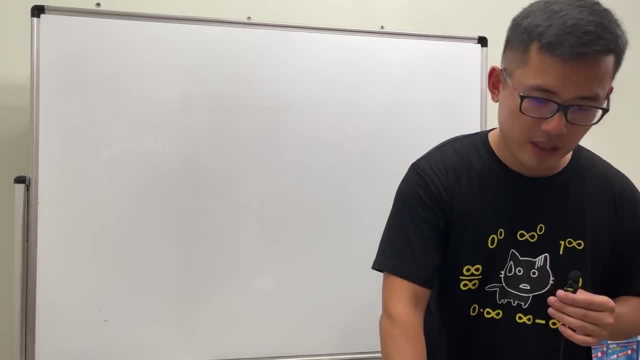 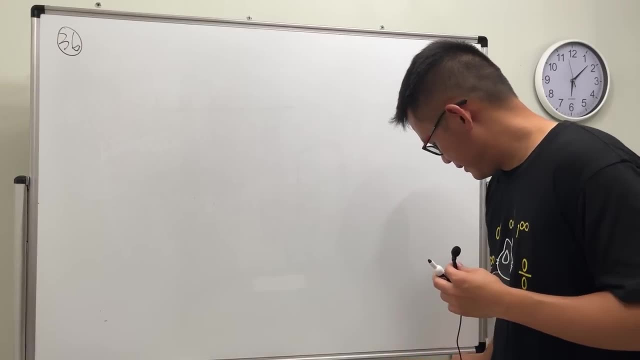 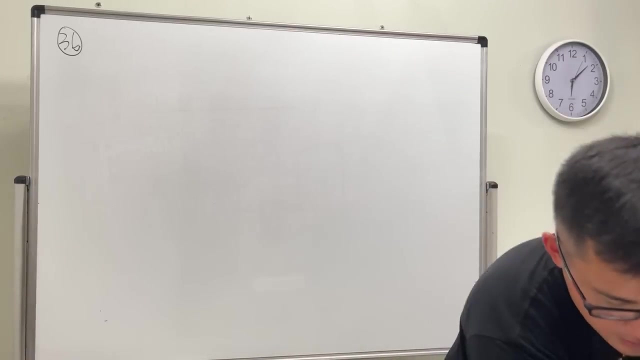 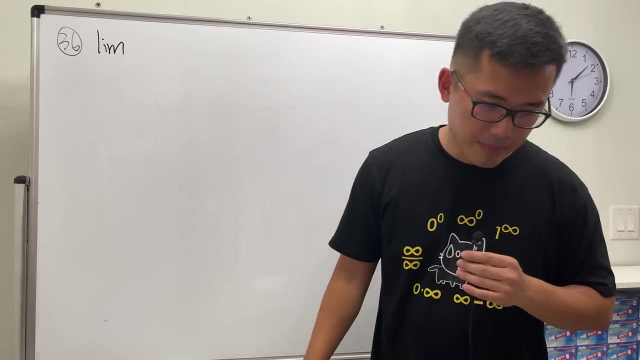 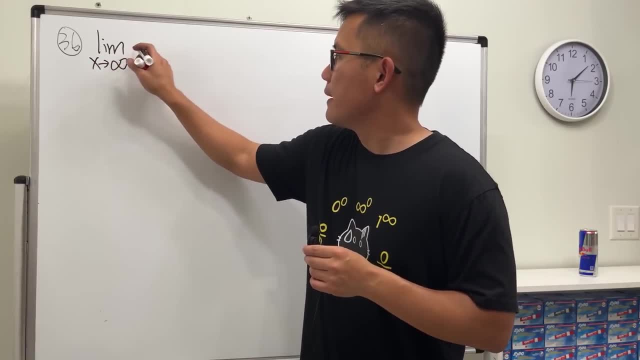 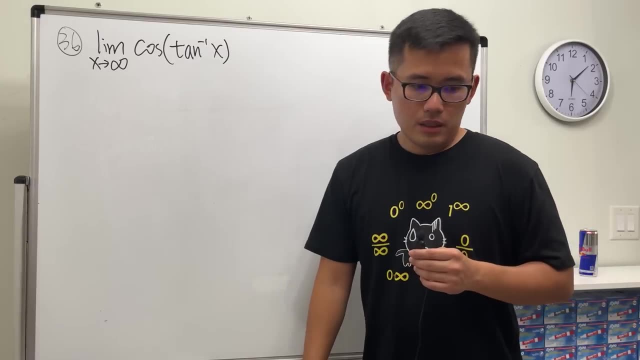 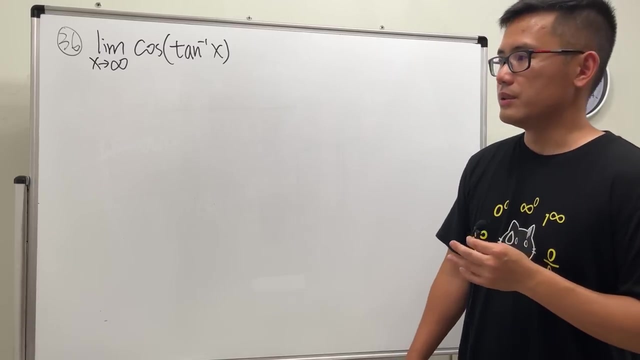 we have x approaching infinity and then we have cosine of inverse tangent of x. okay, so for this kind of questions, it really depends on your teacher, your professor, your TA to to see how they want you to show work. this is how I will allow my students, for how I 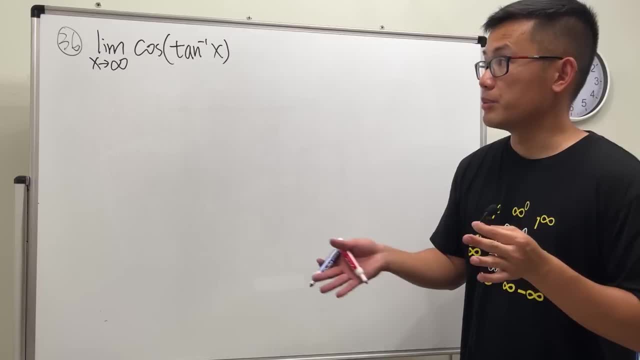 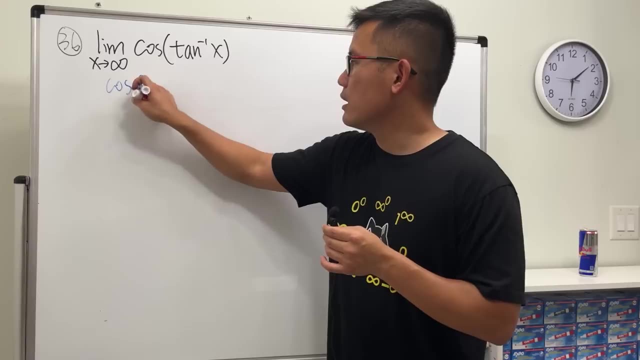 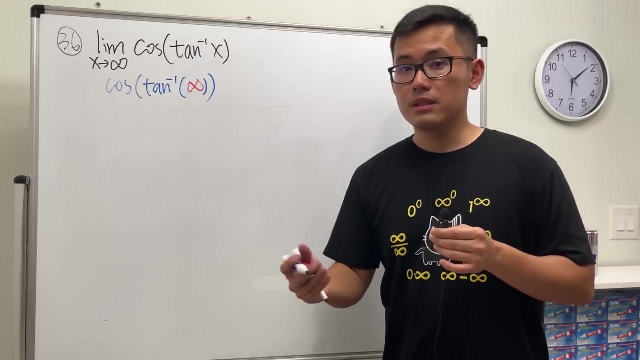 will show work to help students navigate the computation. You can just plug infinity into the x and then just kind of reason it out along the way. so we are going to get cosine of inverse tangent of infinity and just have to remember that we're taking a limit. so then that will be okay and then just draw arrows because 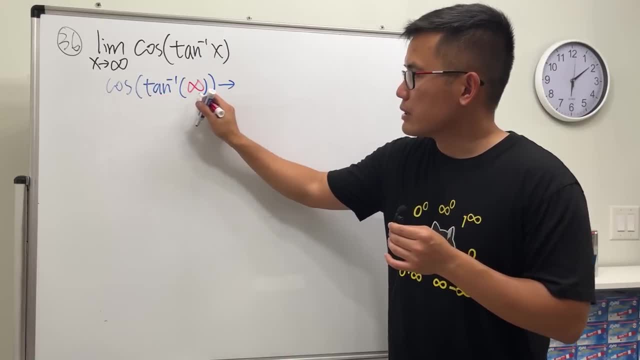 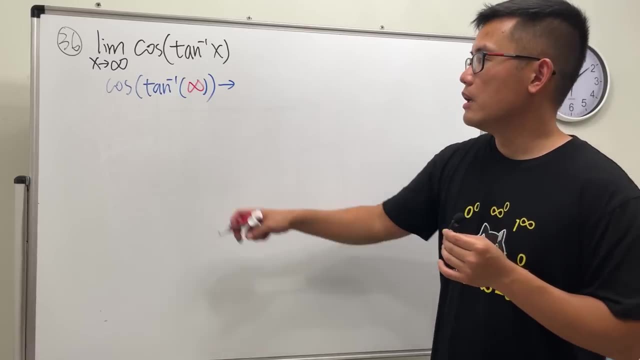 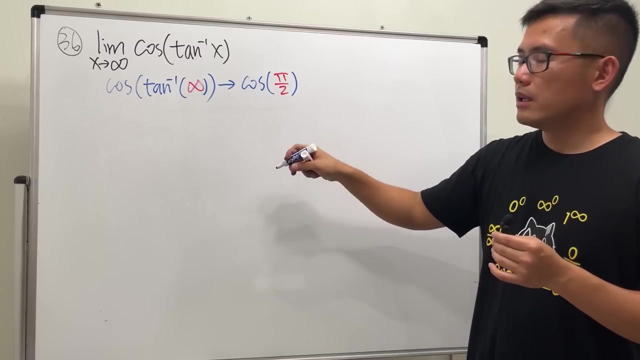 you are taking a limit, So inside out inverse tangent of infinity, meaning the limit as x approaching infinity of inverse tangent. the inside here gives us pi over 2, so we have cosine of pi over 2, and this is nice because cosine of pi over 2, nice and sweet and nice right, sure. 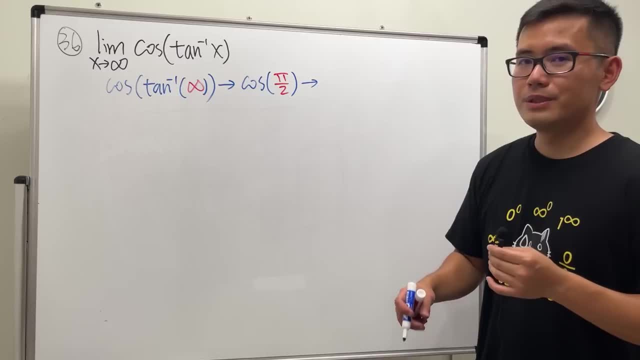 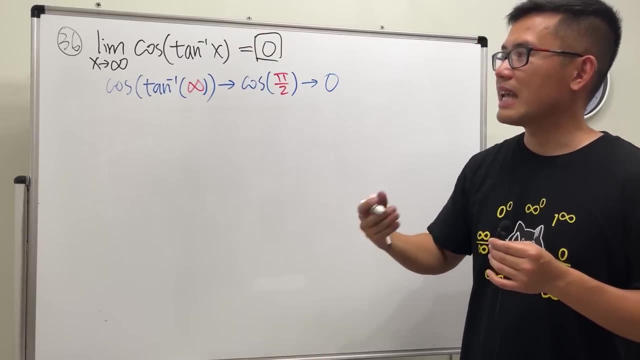 that's sweet. what's cosine of pi over 2,, 0, yeah, so the answer for this right here is just 0.. We're done just inside out, inside out, and of course, for this kind of questions. 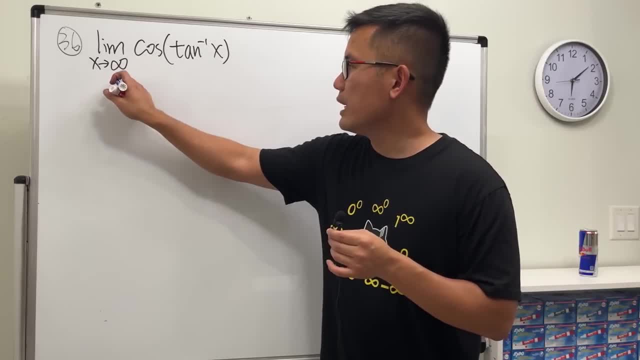 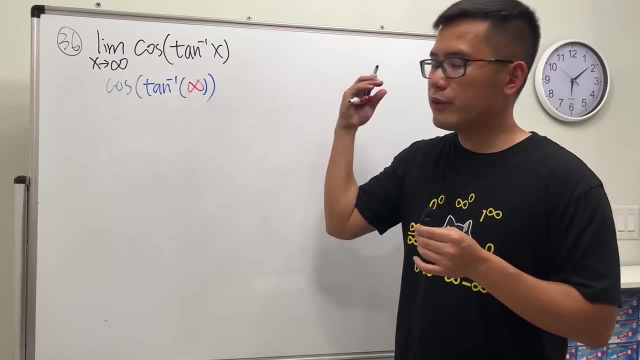 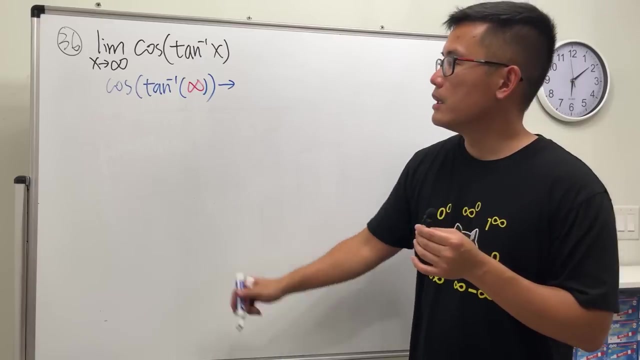 infinity into the X and it just kind of recently out a long way. so we are going to get cosine of inverse tangent of infinity and just have to remember that we're taking a limit. so then that will be okay, and then just draw arrows because you are taking a limit. so inside out, inverse tangent of infinity meaning. 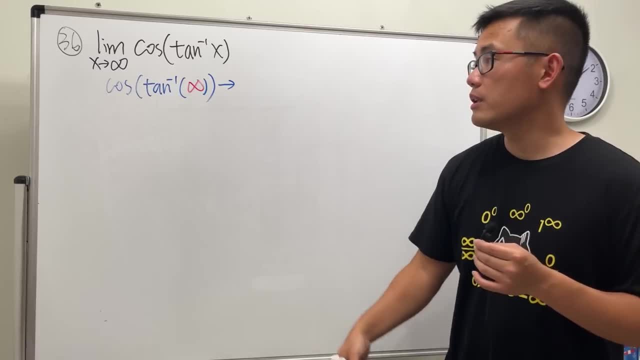 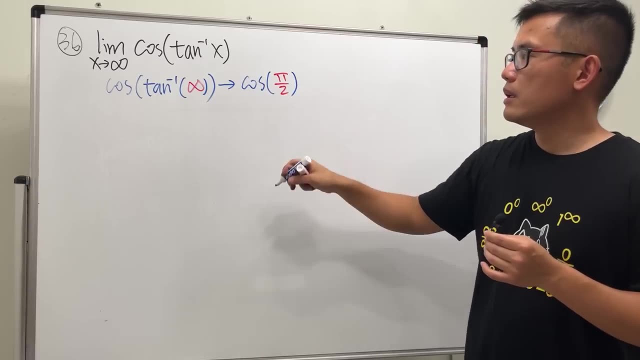 the limit as X approaching infinity of inverse tangent. the inside here gives us pi over 2, so we have cosine of inverse tangent of infinity, so we are going to cosine of pi over 2 and this is nice, because cosine of pi over 2, nice, and 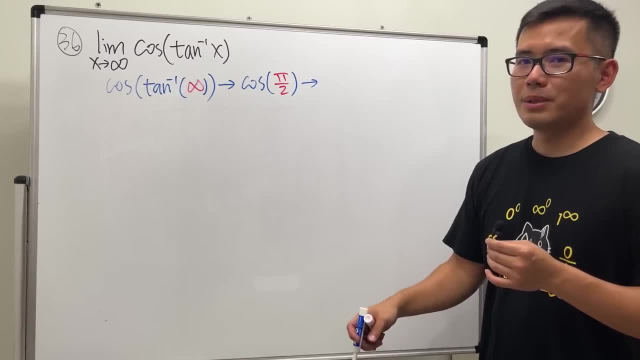 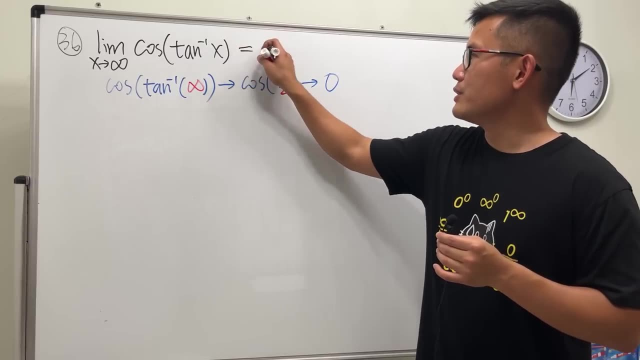 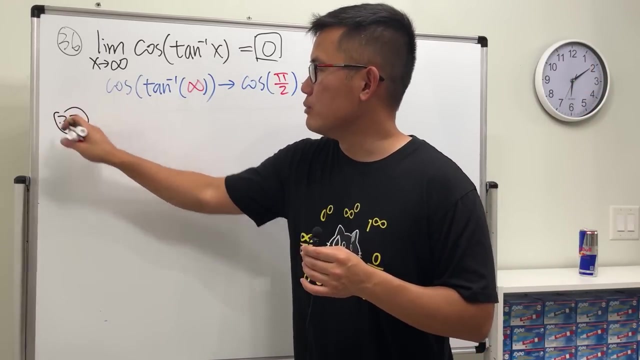 sweet and nice, right, short and sweet. what's cosine of pi over 2, 0? yeah, so the answer for this right here is just 0, and then we are done just inside out, inside out, and of course, for this kind of questions you will have to remember the. 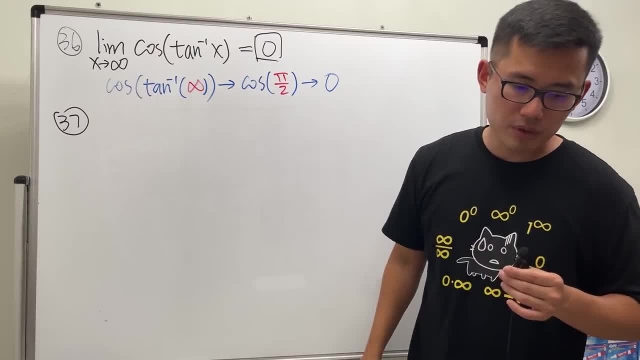 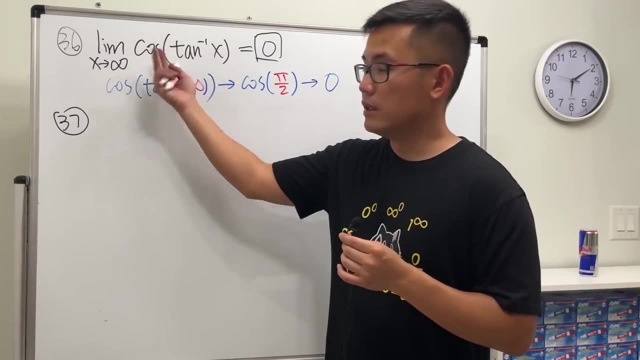 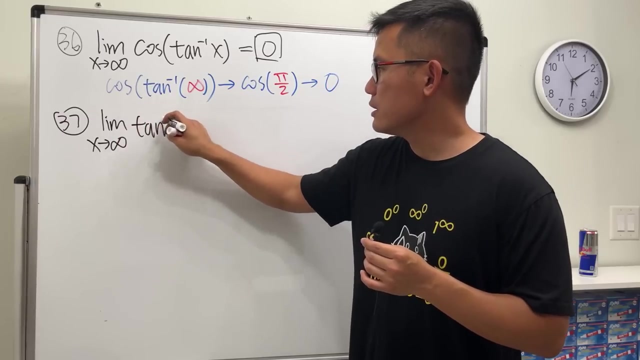 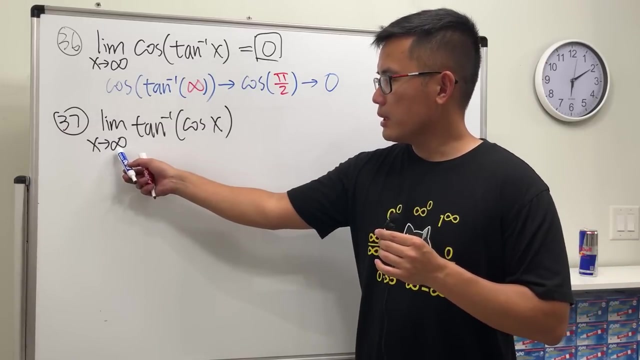 limit as X approaching infinity, like the things I told you guys on the first page. use the graph or the special function. you know that, number 37. switch this a little bit. limit X approaching infinity. inverse tangent of cosine of X. well, can we plug infinity into cosine X? what's this if we 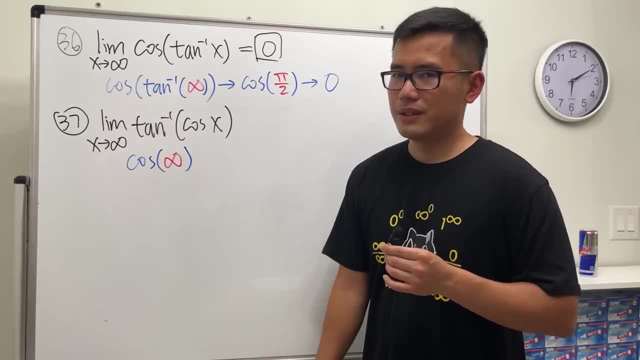 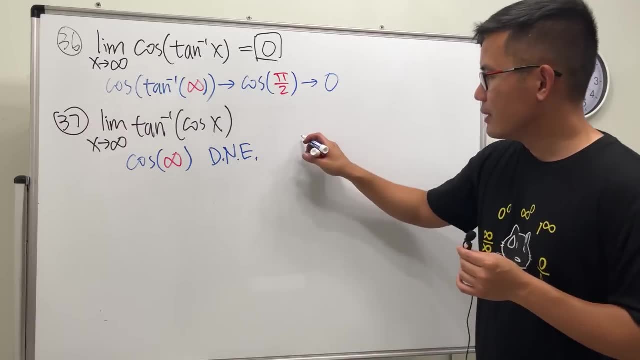 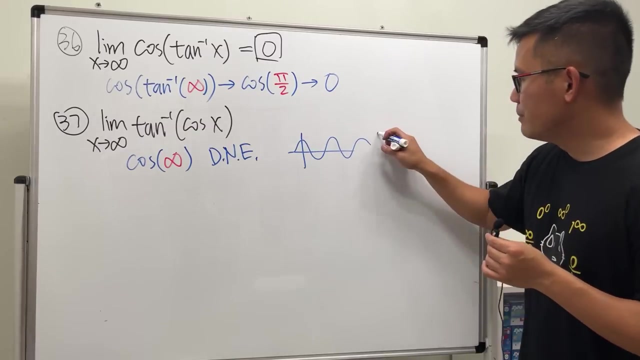 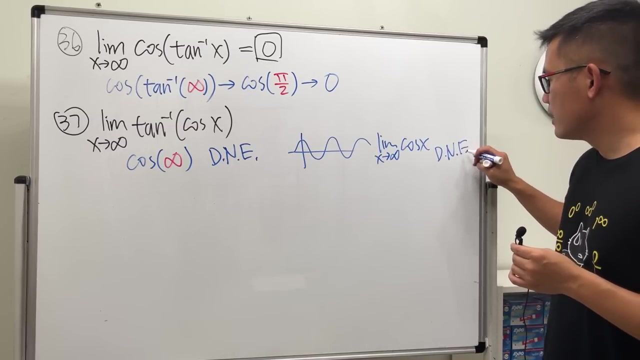 cosine of infinity. what does this mean? this right here does not exist. why? because remember, cosine looks like what right? so the limit as X approaching infinity of cosine X, this right here is just D and E. all right done. if the inside is D and E already, you don't need to worry about what's after. this is not possible. 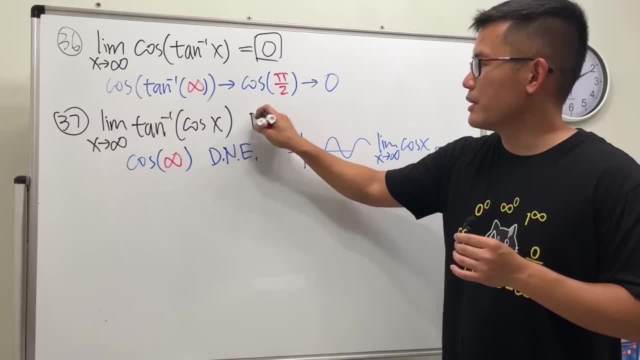 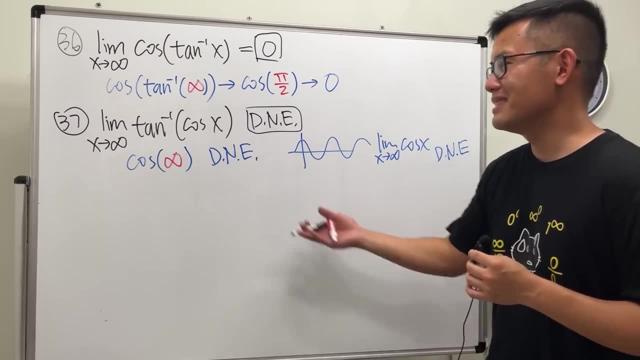 already. you don't need to worry about what's after. this is not possible to do so. this radius D and E, it's not cause. inverse tangent of D and E is D and E you kind of like that. i don't do, that did. this is number 38. everybody will love this kind. 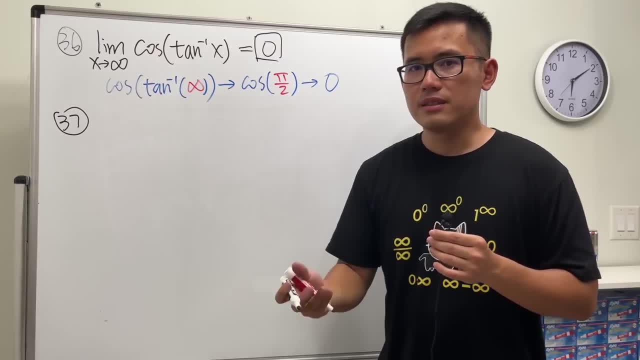 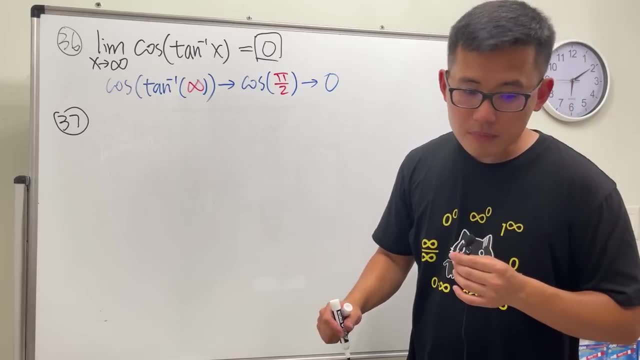 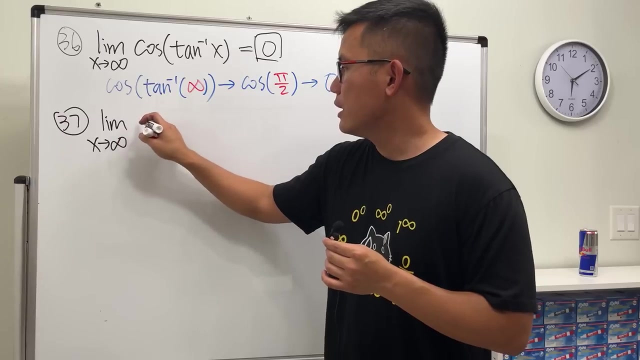 you will have to remember the limit as x approaching infinity, like the things I told you guys on the first page. use the graph or the special function and all that Number 37, I'll switch this a little bit: limit x approaching infinity- inverse tangent. 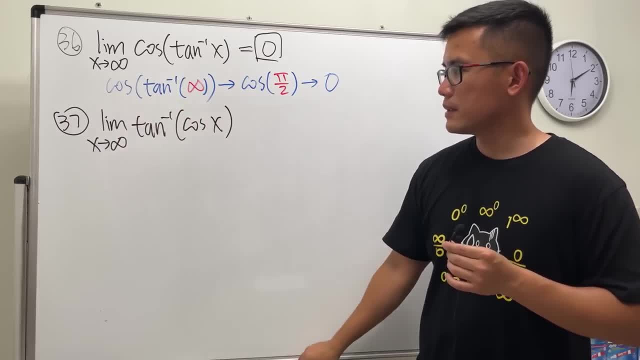 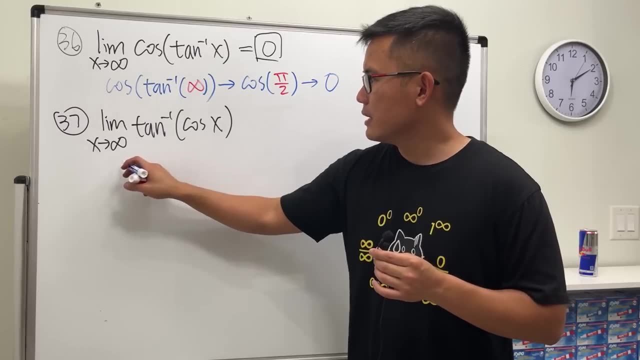 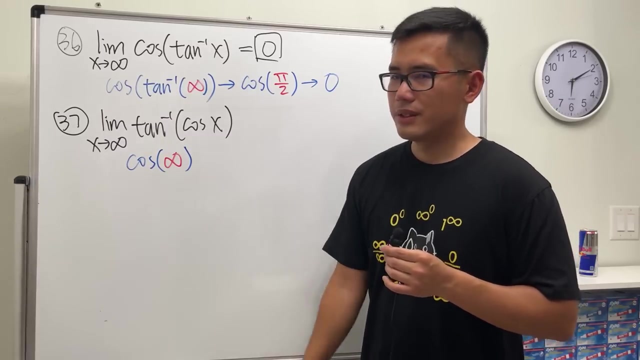 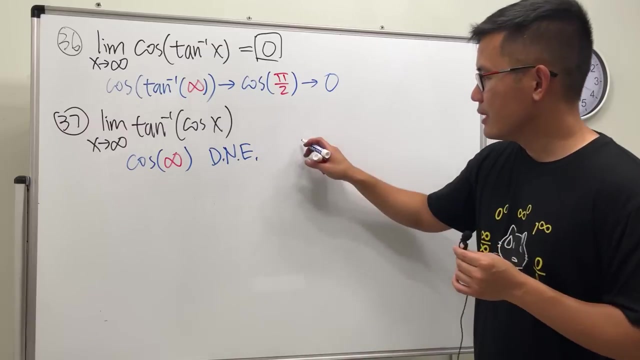 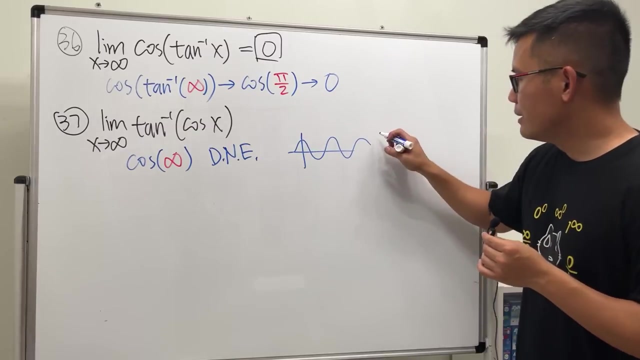 of cosine of x. Well, can we plug infinity into cosine x? What's this? If we cosine of infinity, what does this mean? This right here does not exist. why? Because remember, cosine looks like what right. so the limit as x approaching infinity of. 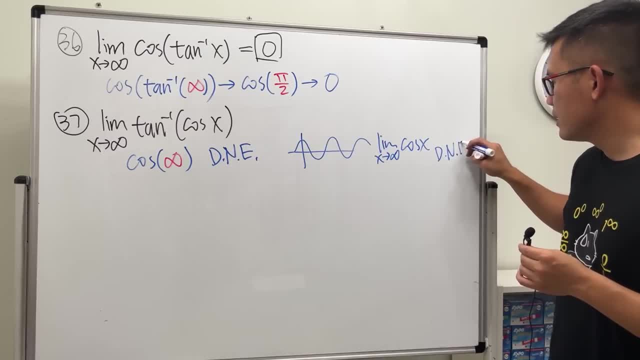 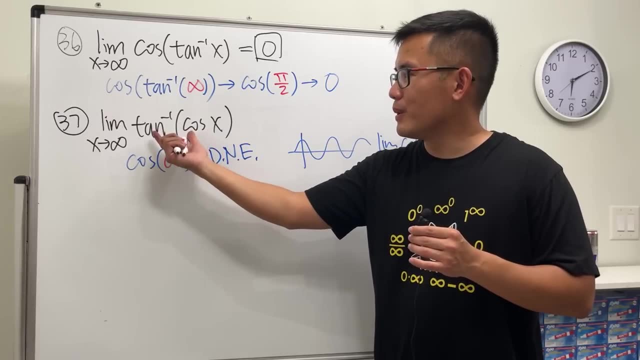 cosine x. this, right here, is just d and e. all right done. If the inside is d and e already, you don't need to worry about what's after. this is not possible to do, so this, right here, is d and e. 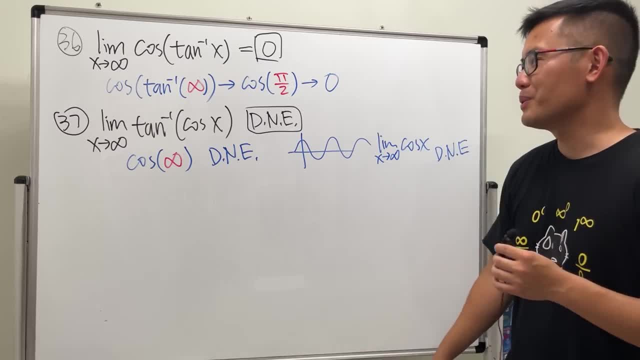 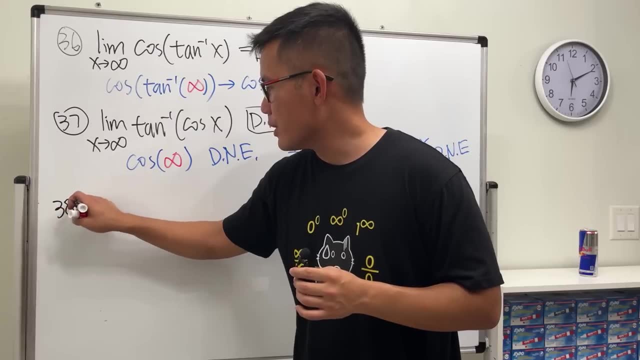 It's not because the inverse tangent of d and e is d and e, kind of like that. but don't do that. this is much better that way. Number 38, everybody will love this kind of question. Limit as x approaching infinity. 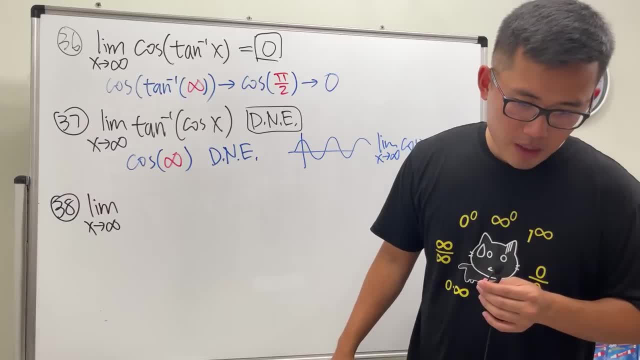 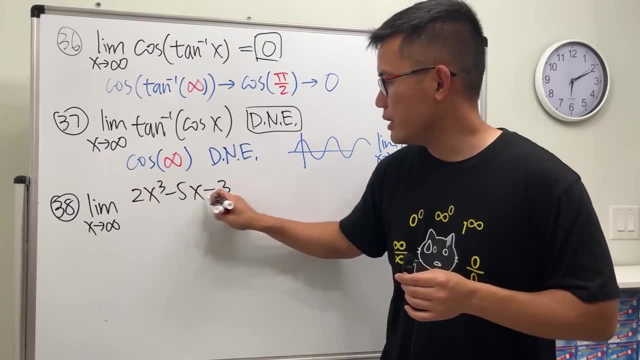 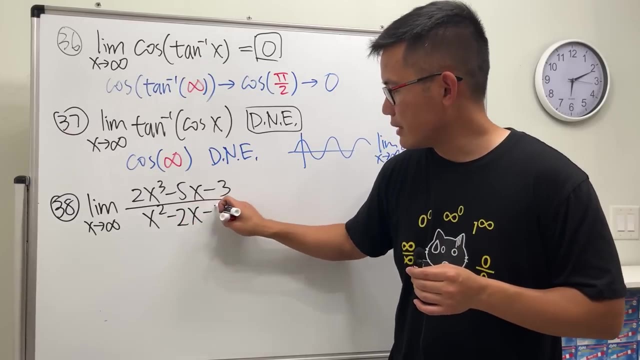 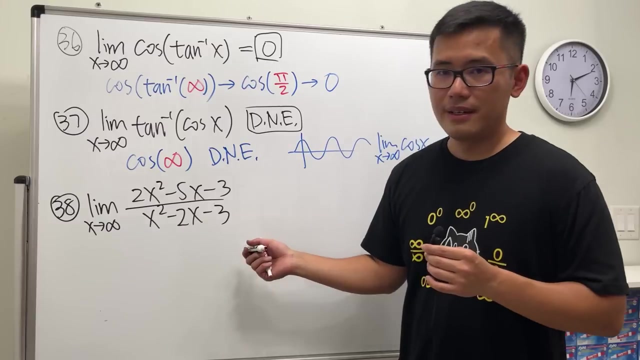 We have 2x to the third power, minus 5x, minus 3, over, oh, x squared minus 2x, minus 3, sorry, this right here meant to be square. Does this look familiar? It should, huh. 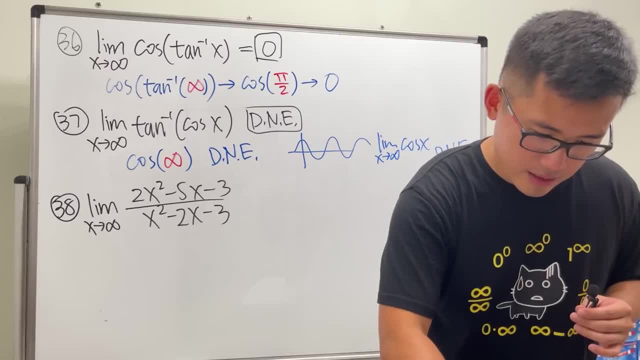 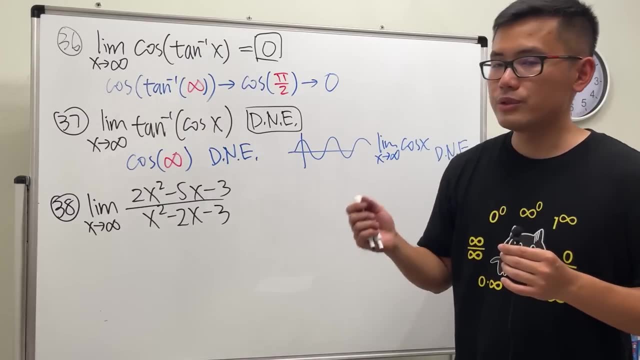 Is that? yeah, Okay, It's number 22,, isn't it? Except for the fact that for number 22, it was x approaching 3, but right now it's x approaching infinity, When we have x approaching infinity much easier. 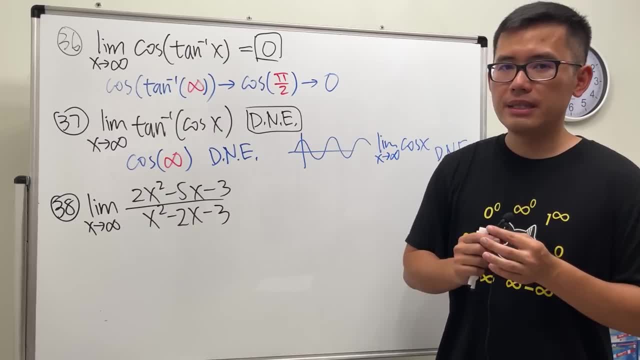 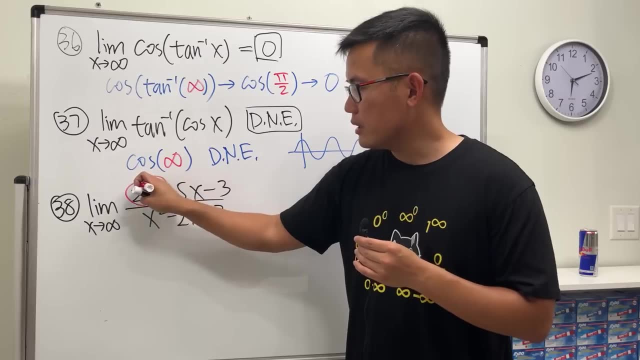 We just have to care about the dominating part on the top and also the dominating part on the bottom. In this case, we just have to worry about the biggest power of x on the top, which is 2x squared on the bottom. we just have to worry about the x squared. 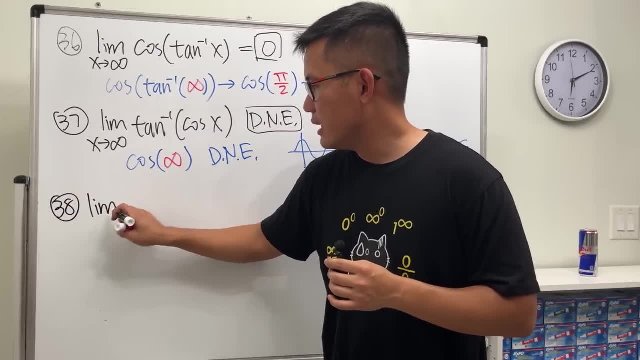 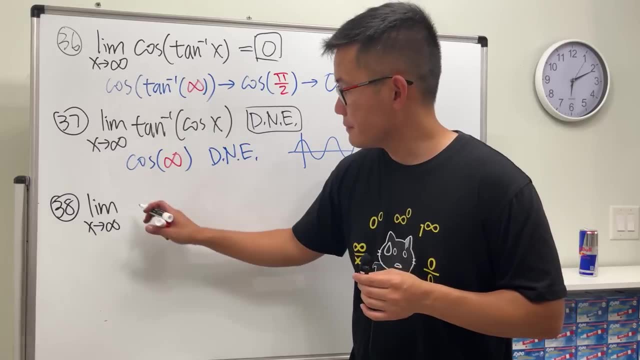 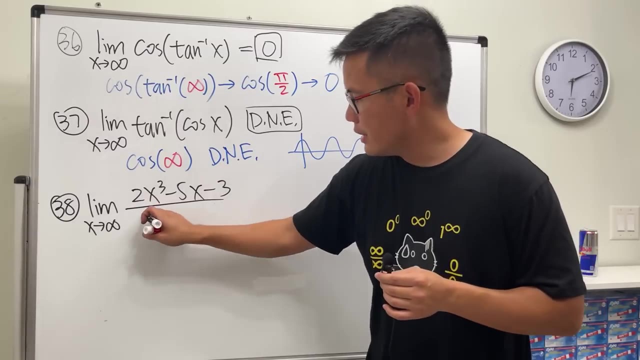 of question limit. as X approaching infinity, we have 2X to the third power minus 5, X minus 3 over Oh, x squared minus 2x minus 3.. Sorry, this is what you meant to be. It's a square. 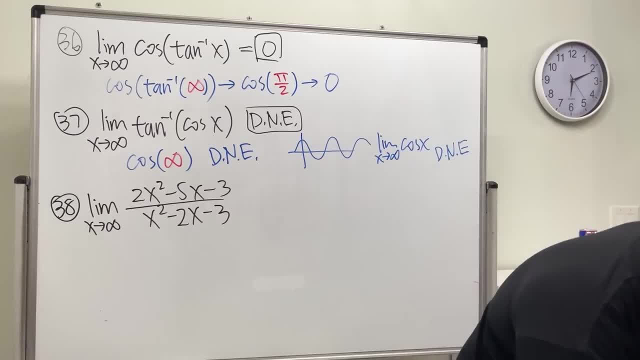 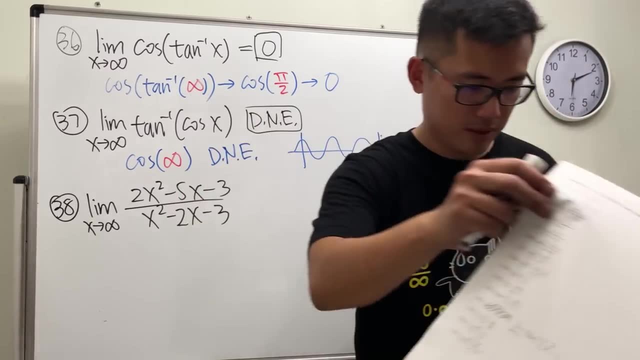 Does this look familiar? It should huh, Is that? Yeah, It's number 22,, isn't it? Except for the fact that for number 22, it was x approaching 3. But right now it's x approaching infinity. 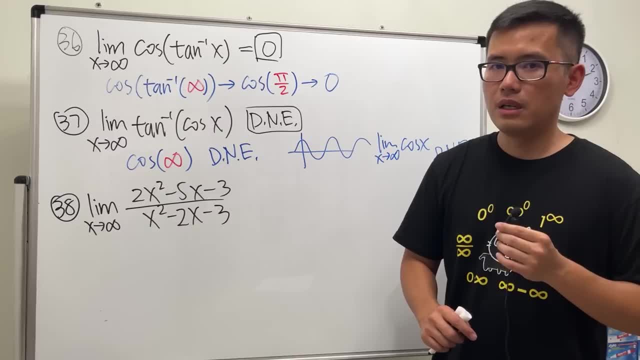 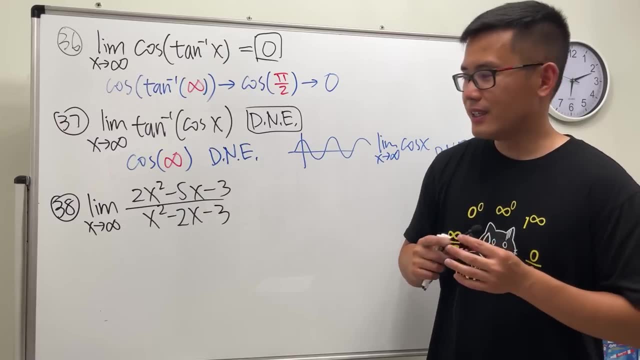 When we have x approaching infinity, it's much easier. We just have to care about the dominating part on the top and also the dominating part on the bottom. In this case, we just have to worry about the biggest power of x on the top, which is 2x squared. 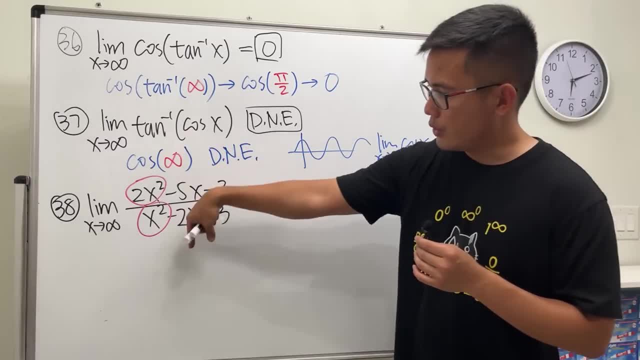 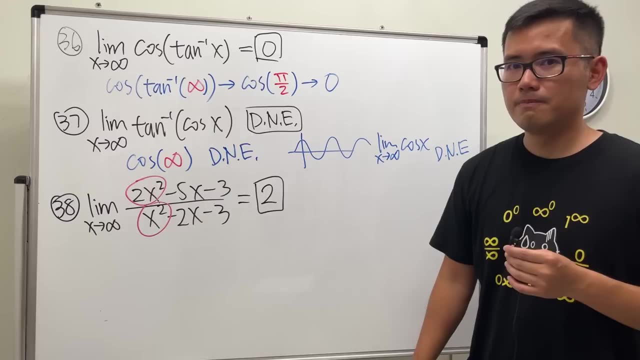 On the bottom. we just have to worry about the x squared Reduce. we get 2, and then we are done. This is the limit that you do not want to miss. Alright, why does this work? I'm going to show you. 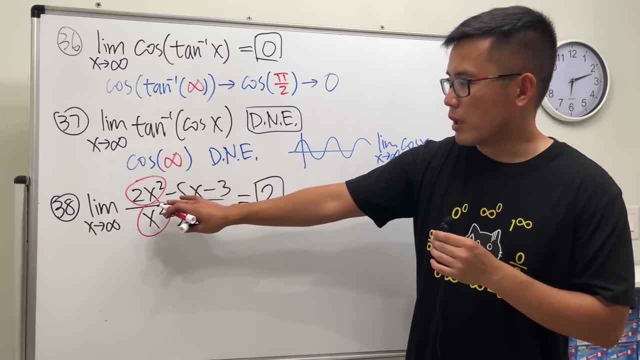 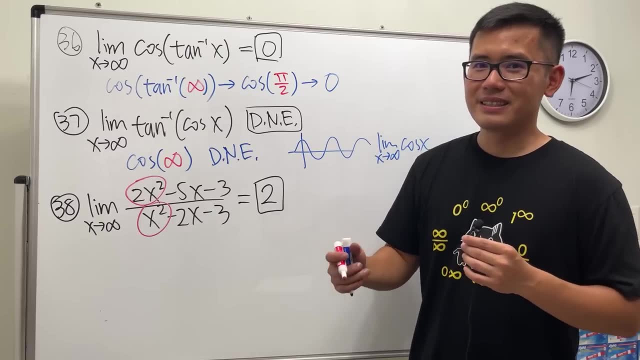 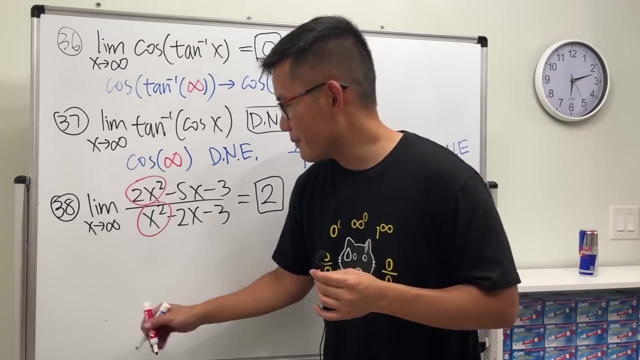 I just want to make a remark first, though. If you are taking my class, if you do this, I'm totally cool with that, But if you are taking a class with a different professor, if your professor wants you to do the following, then just do it this way. 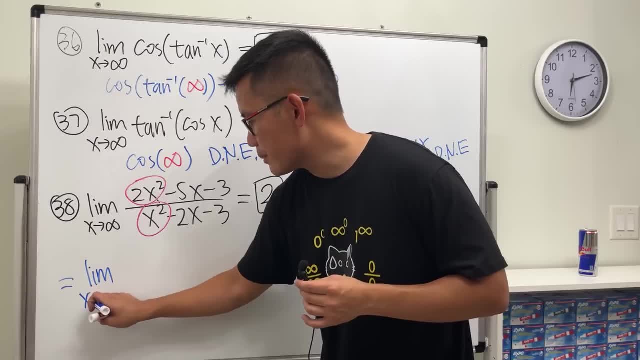 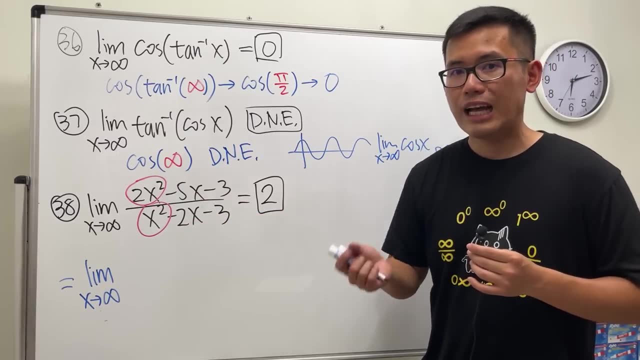 Here's the deal: When we are taking the limit as x approaching infinity- and keep in mind, this is x approaching infinity. that's why we didn't even need to bother to factor whatsoever, We just had to pick down the dominating When we have x approaching infinity. let me write this down again: 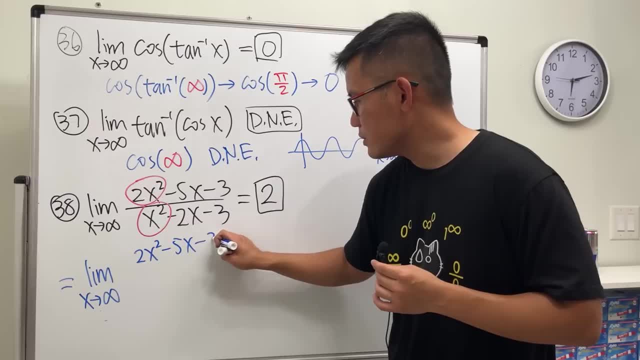 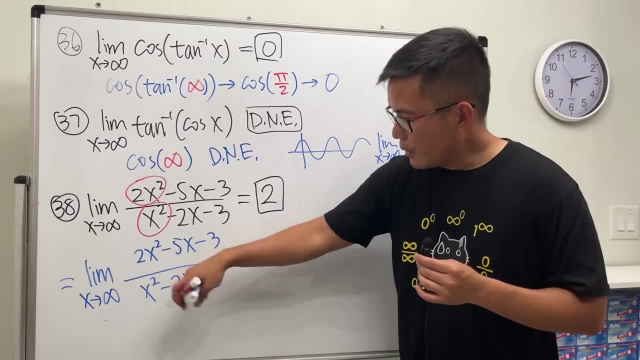 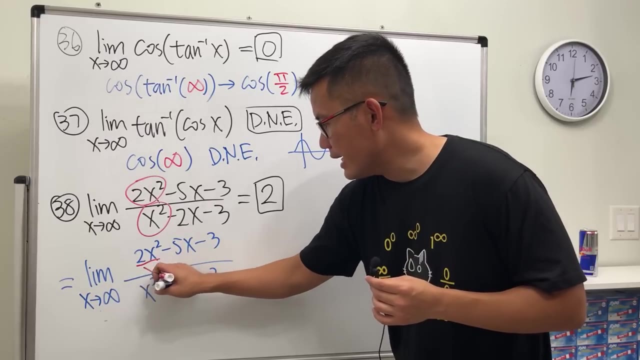 We have 2x squared minus 5x minus 3 over x squared minus 2x minus 3.. When we have this, look at the biggest power of x, and that is x squared, And what you want to do is divide everybody by x squared. 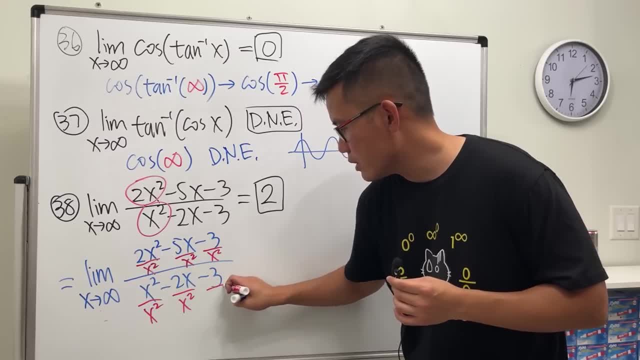 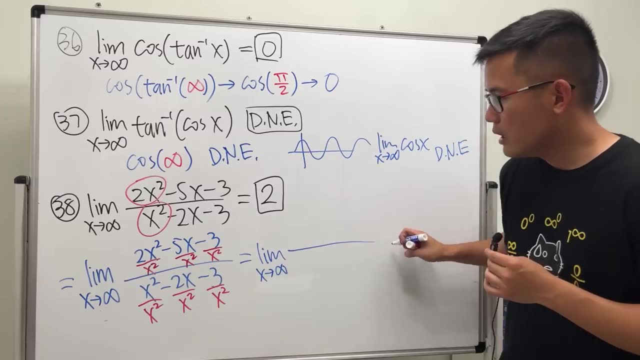 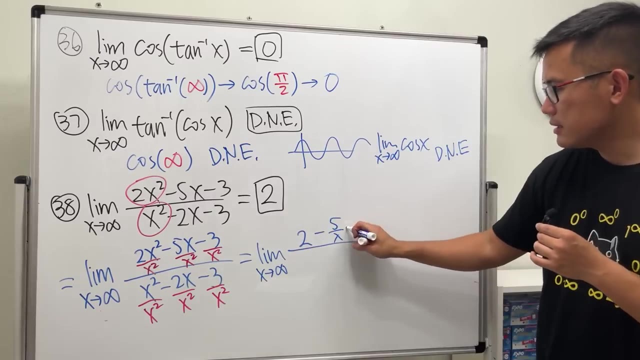 Divide everybody by x squared And once we do that, we are looking at the limit as x approaching infinity. This is out, It's just a 2.. But then we will have minus 5 over x and then minus 3 over x squared. 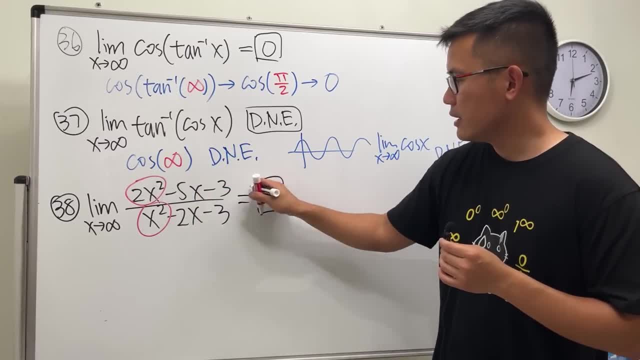 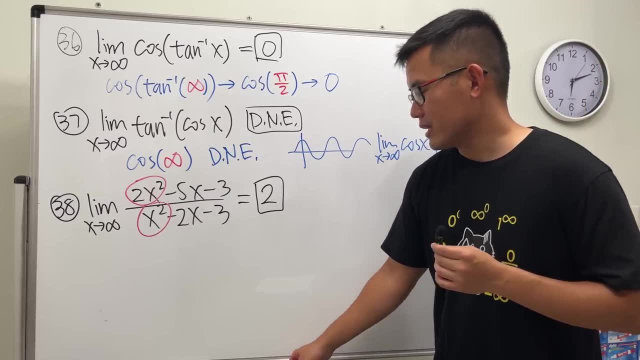 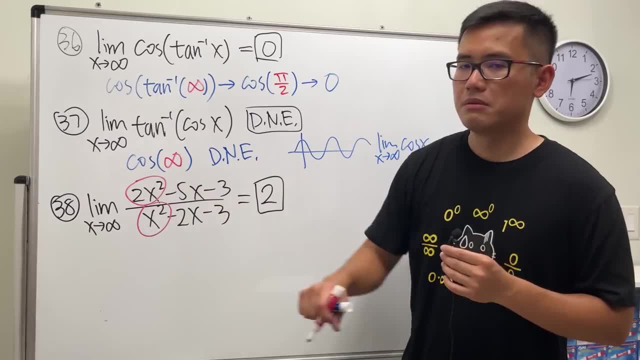 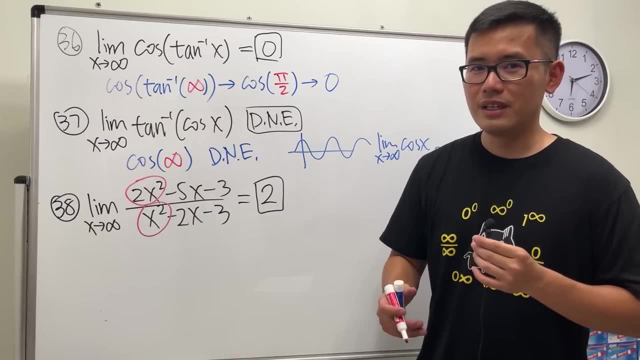 I just want to make a remark first, though. If you are taking my class, if you do this, I'm totally cool with that, But if you are taking a class with a different professor, if your professor wants you to do the following, then just do it this way. 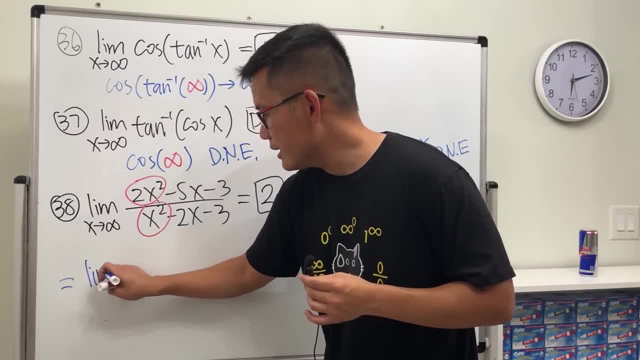 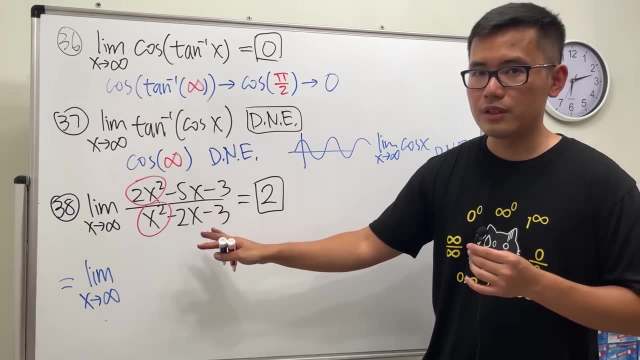 Here's the deal. There's this. No, There's this, guys taking the limit as x approaching infinity. and keep in mind, this is x approaching infinity. that's why we didn't even need to bother to factor whatsoever. we just had to pick out the dominating. 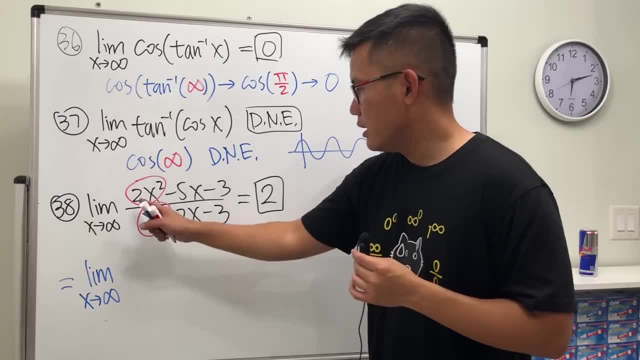 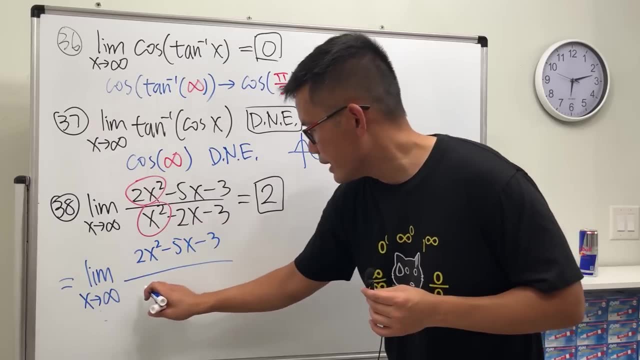 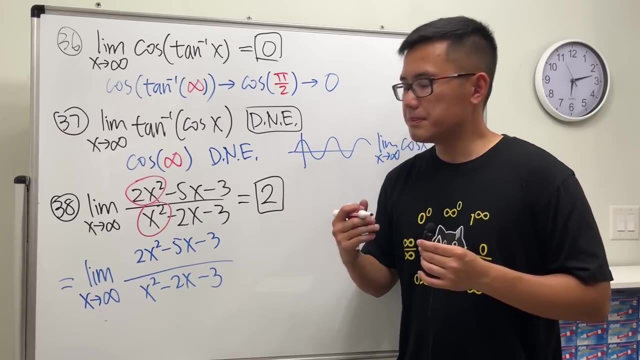 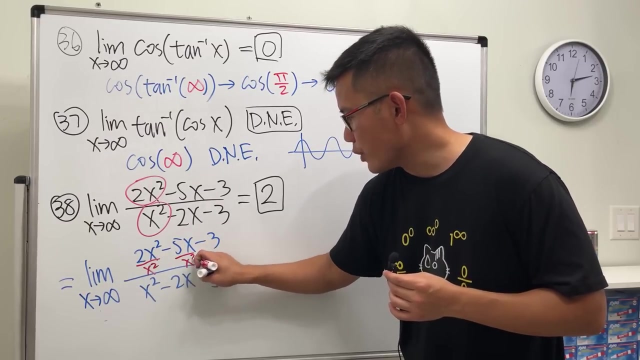 part, when we have x approaching infinity. let me write this down again: we have 2x squared minus 5x minus 3 over x squared minus 2x minus 3.. when we have this, look at the biggest power of x, and that is x squared, and what you want to do is divide everybody by x squared. 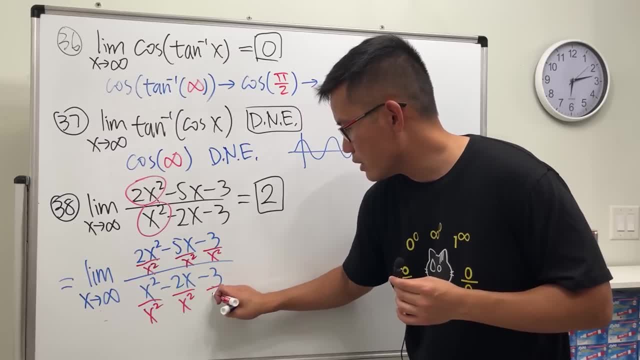 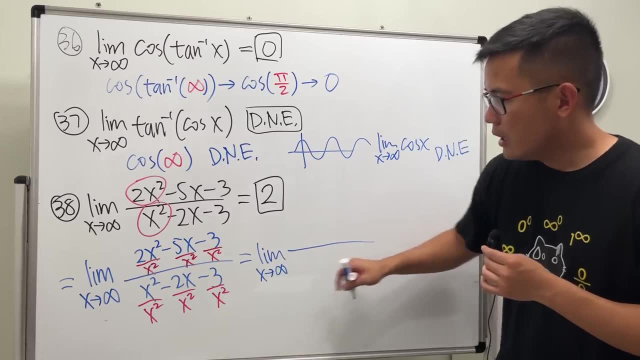 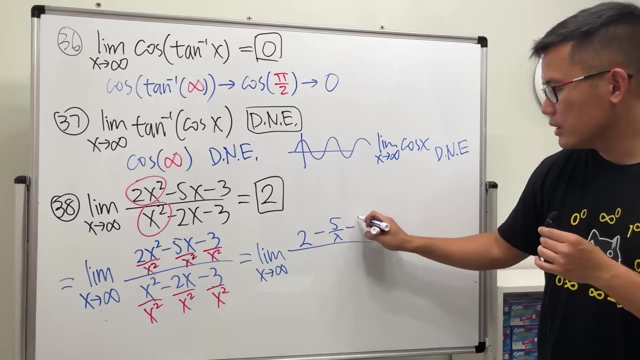 divide everybody by x squared, and once we do that, we are looking at the limit as x approaching infinity. this is out, it's just a 2, but then we will have minus 5 over x, and then minus 3 over x squared, and then that will be just 1. 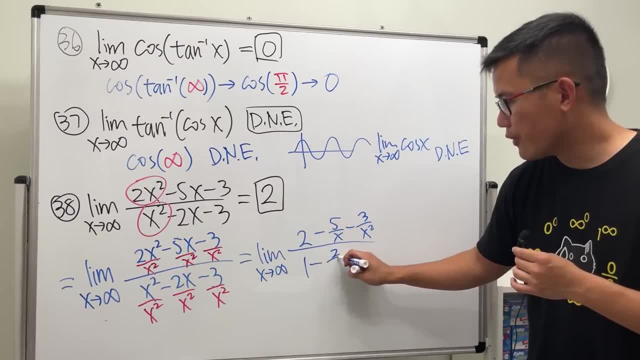 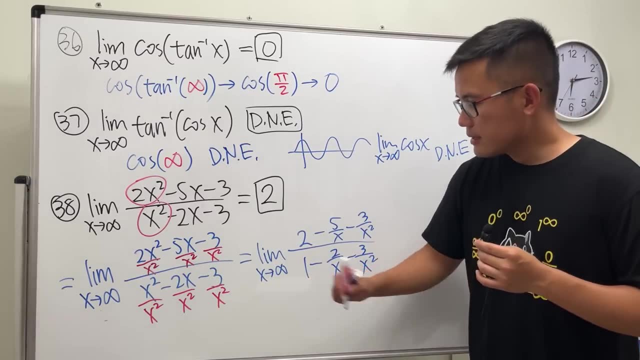 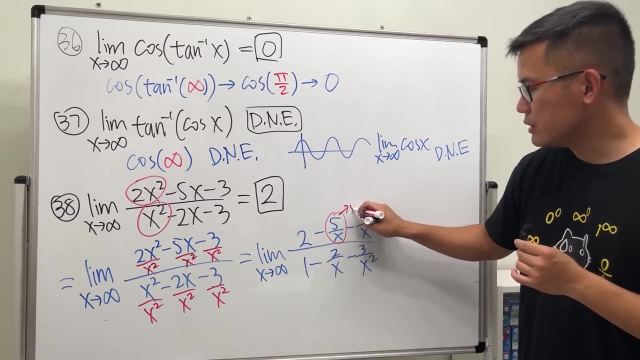 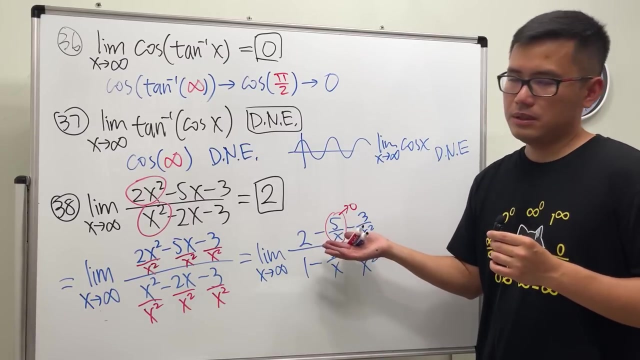 and the minus, that is, 2 over x. and then lastly, minus 3 over x, square as x goes to infinity. this has no x, so it has to be 2, but 5 over x. this will approach 0, because we discussed this before. 5 over infinity will approach 0, even though it's a minus. minus, just 0. 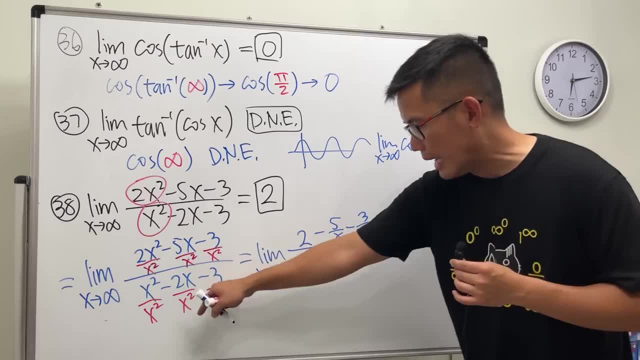 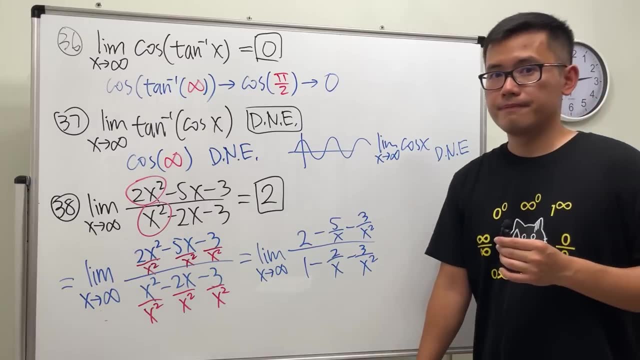 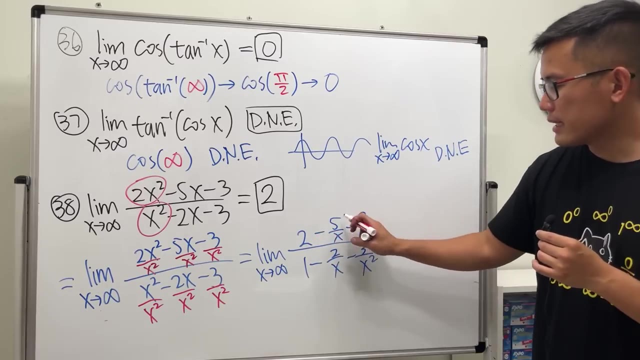 And then that will be just 1.. And then minus, that is 2 over x. and then, lastly, minus, 3 over x, squared As x goes to infinity. this has no x, so it has to be 2.. But 5 over x. this will approach 0, because we discussed this before. 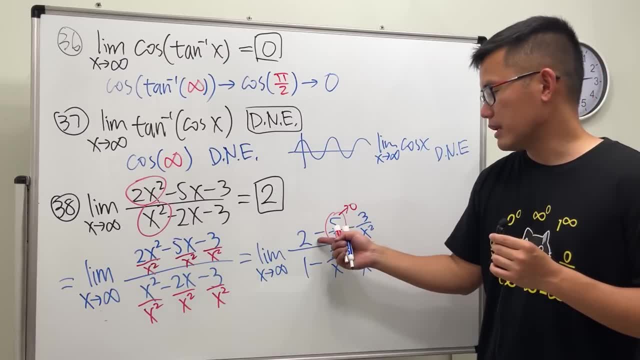 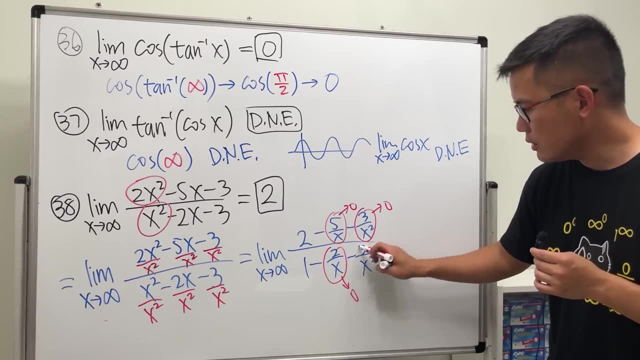 5 over infinity will approach 0,. even though it's a minus, it's just 0.. Similarly, this will also approach 0, likewise 0, likewise 0. In other words, these parts, they don't really matter. 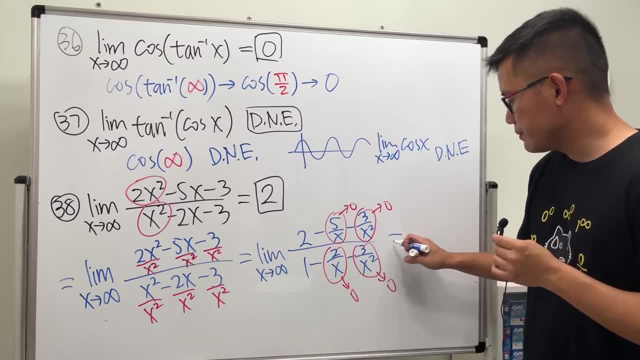 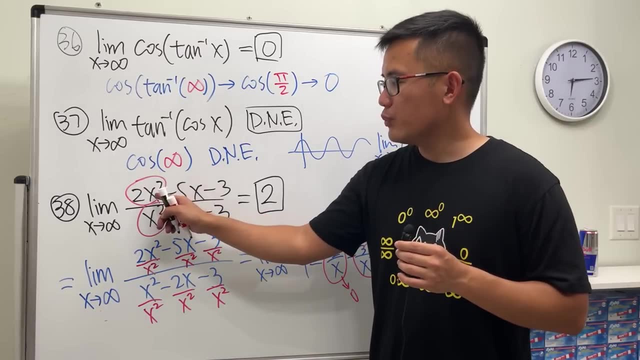 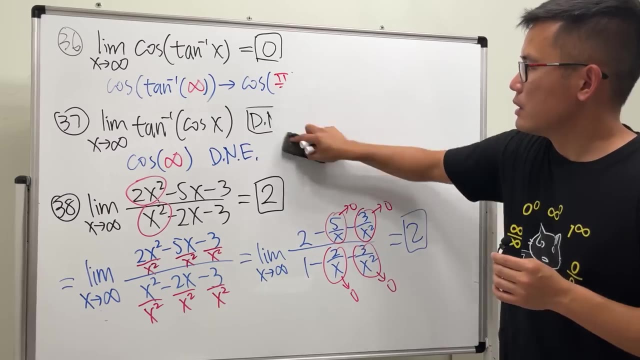 It's just a 2 and also the 1.. Reduce that, we get 2.. Reduce that. However, if the power on the top, let's say we have x plus 3 power, Let me just probably give you guys like a small bonus on the side. 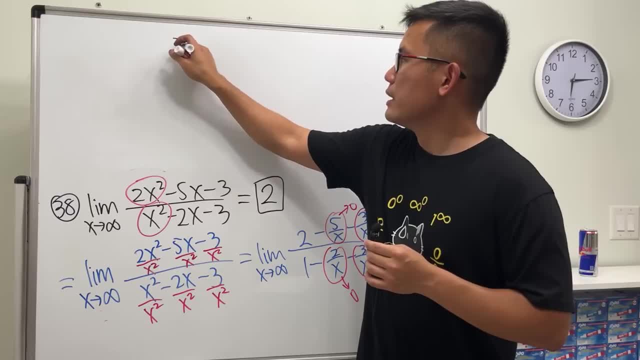 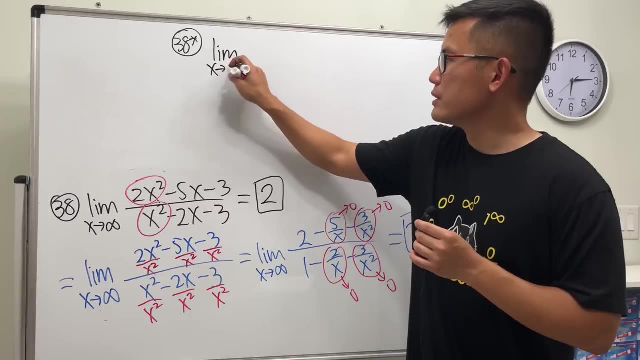 Before we continue, that's number 38.. So number 38 with a star next to it, just like a small variation, If we have the limit as x approaches infinity, if we have 2x to the third power, and then minus 5x, minus 3,. 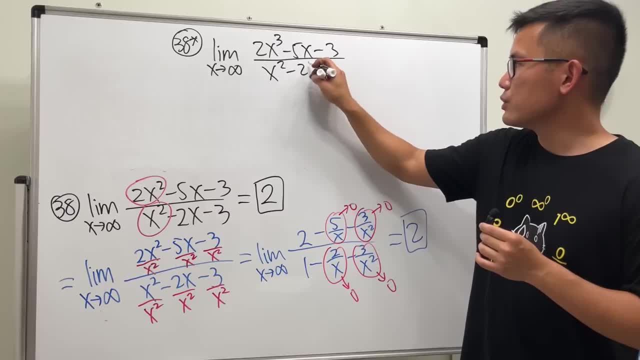 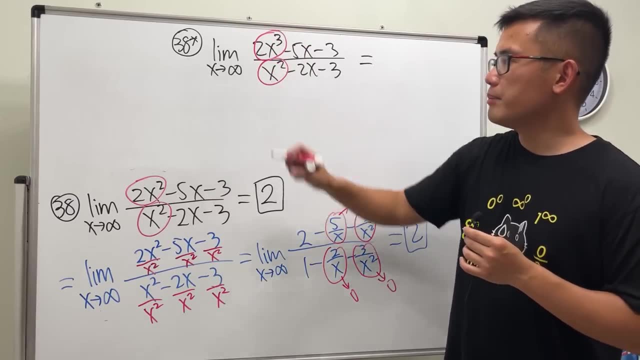 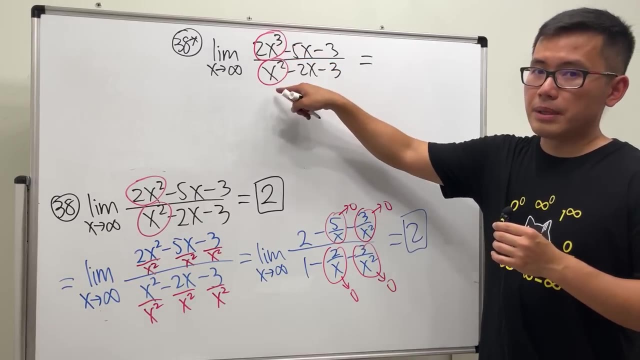 over x squared minus 2x minus 3.. The dominating part on the top is 2x to the third power and the dominating part on the bottom is x squared, the highest power of x. pretty much. You see the degree right here. the power right here is bigger than the bottom. 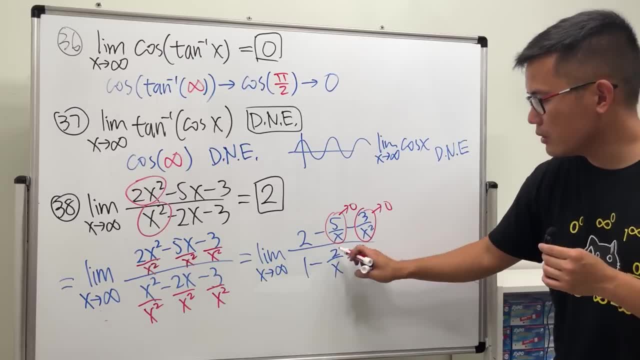 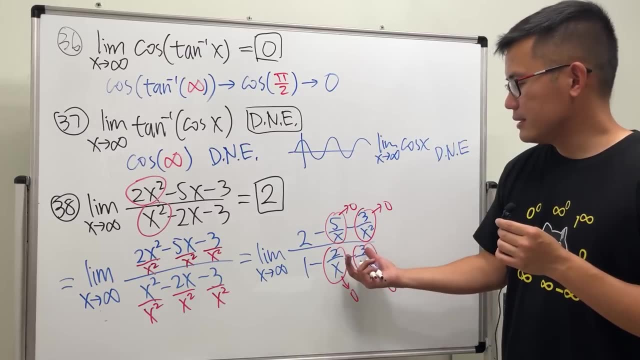 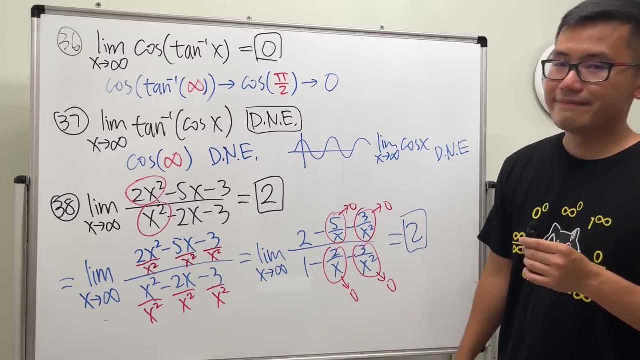 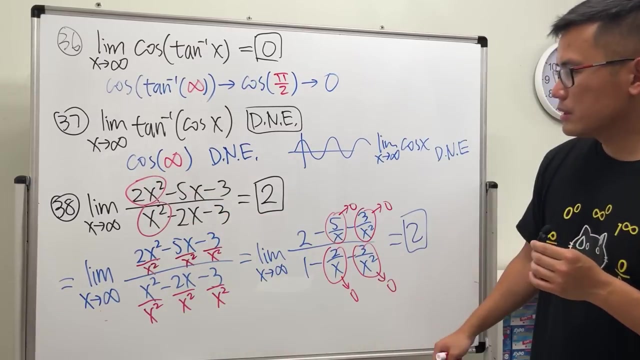 similarly, this will also approach 0, likewise 0, likewise 0. in another word, this part, they don't really matter, it's just the 2 and also the 1 reduce that we get 2 done. however, if the power on the top, let's say we have x plus third power, let me just 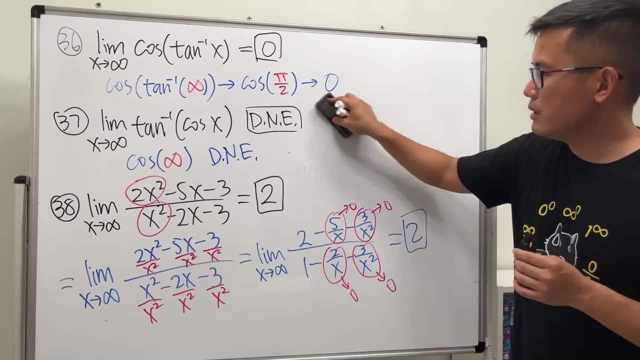 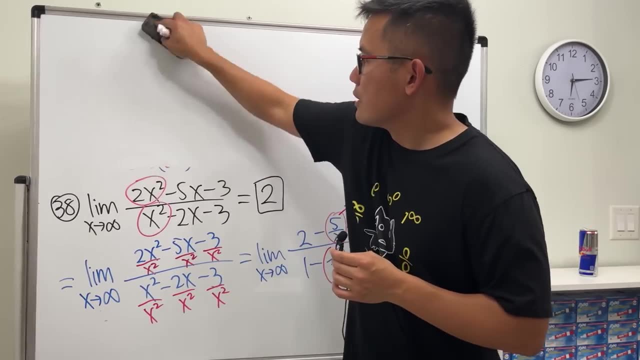 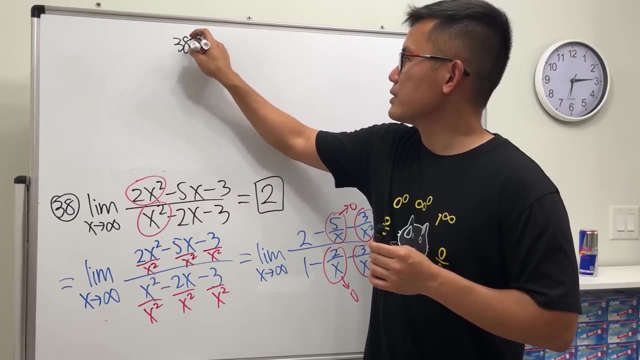 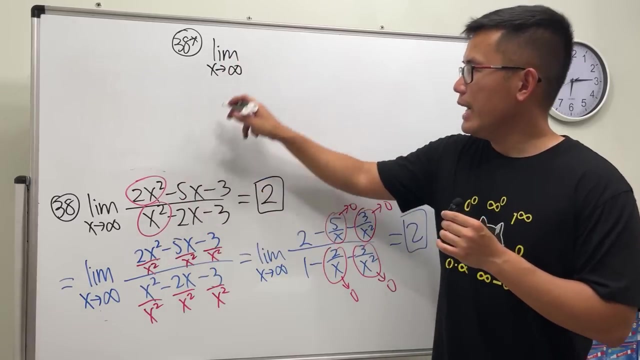 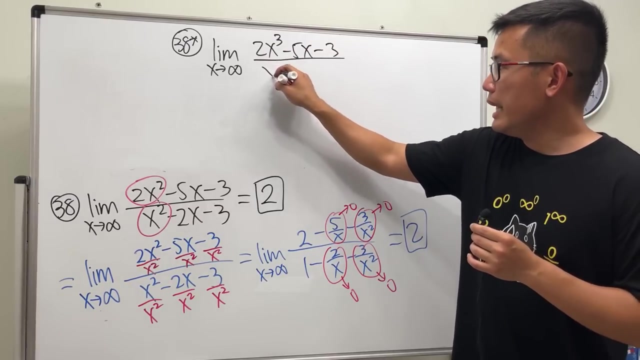 probably give you guys like a small bonus on the side before we continue. that's number 38. so number 38 with a star next to it, just like a small variation. if we have the limit as x approaching infinity, if we have 2x to the third power, and then minus 5x minus 3 over x square, minus 2x minus 3. 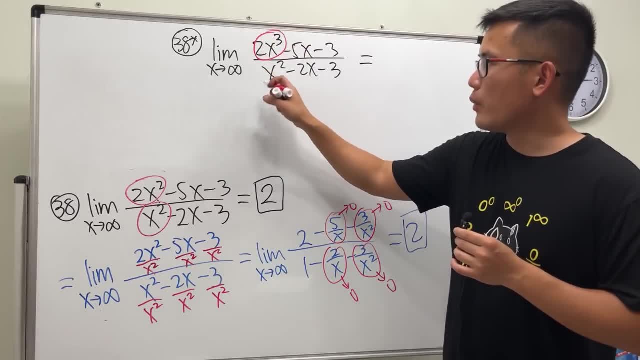 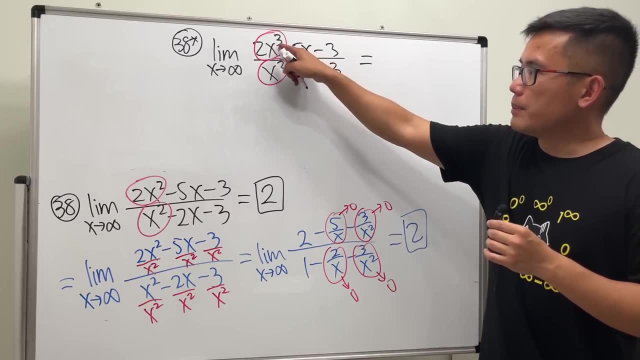 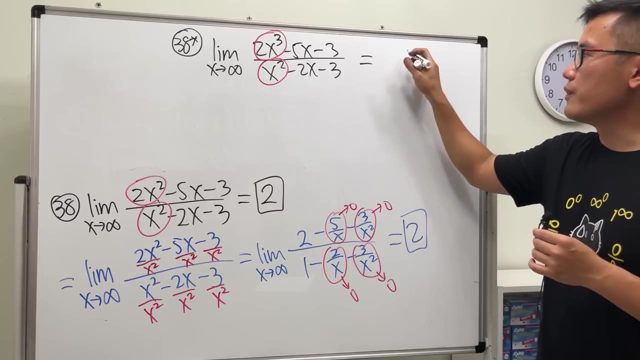 the dominating part on top is 2x plus third power and the dominating part on the bottom is x square, the highest power of x. pretty much. you see that degree right here. the power here is bigger than the bottom. if you reduce you just have x, as x goes to infinity. this right here will go to infinity. 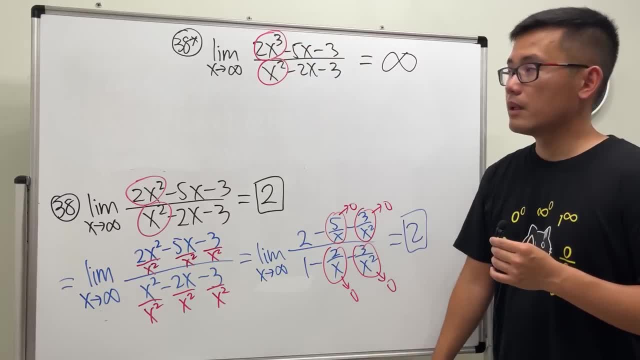 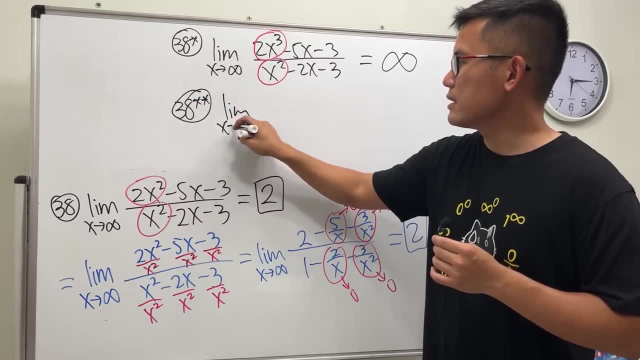 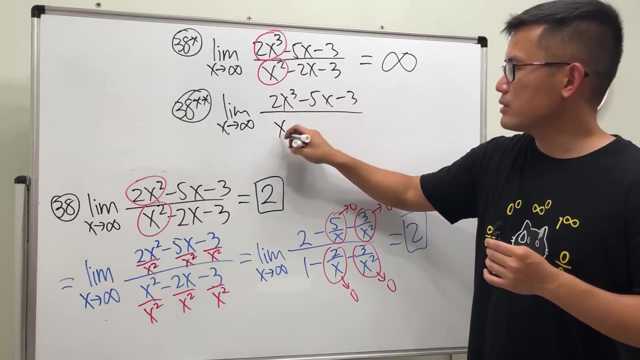 if the degree on the top is bigger, the whole thing goes to infinity. however, number 38, star, star, if we have the limit as x approaching infinity, 2x, let's say third power minus 5x minus 3. but if the bottom is x to the 6th power and then minus 2x, 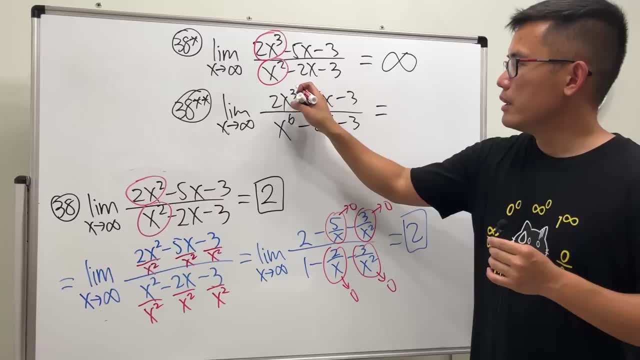 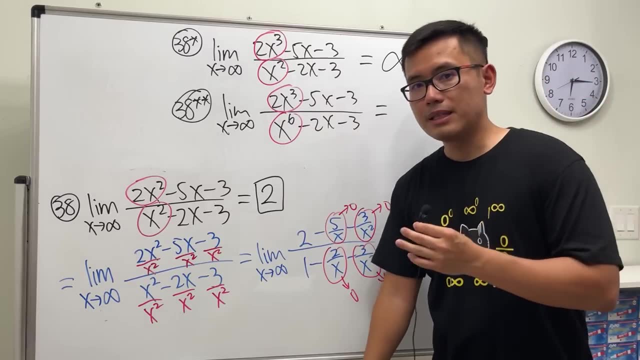 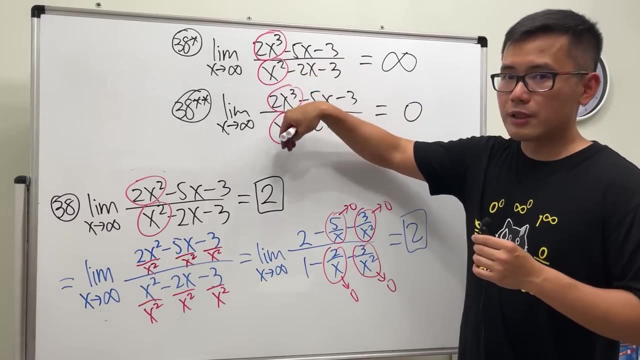 minus 3. you see now the degree on the top is 3. the degree on the bottom here is 6. this is bigger than that. if the bottom is bigger, you get 0 because you can reduce it right. you get 1 over x plus third power. after you reduce, we have 2 over x plus third power. 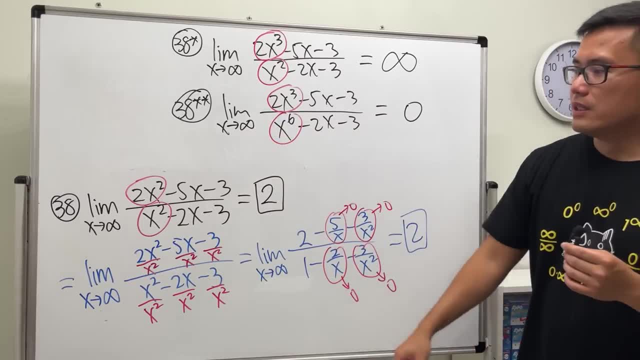 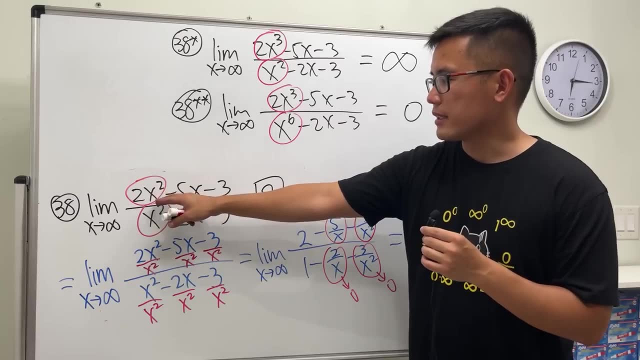 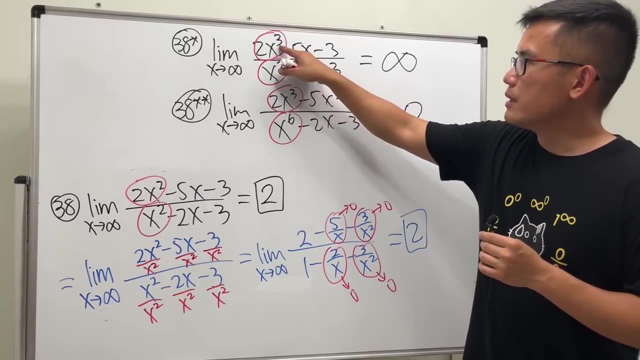 as x total goes to infinity, you get zero. so here are the three situations. you just compare the degree, aka the highest power of x on the top and also on the bottom. if they are the same, reduce the coefficient. if the top is bigger, then the answer will be infinity. if the bottom power right. 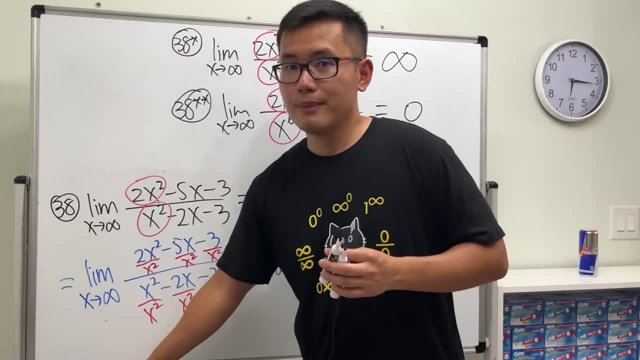 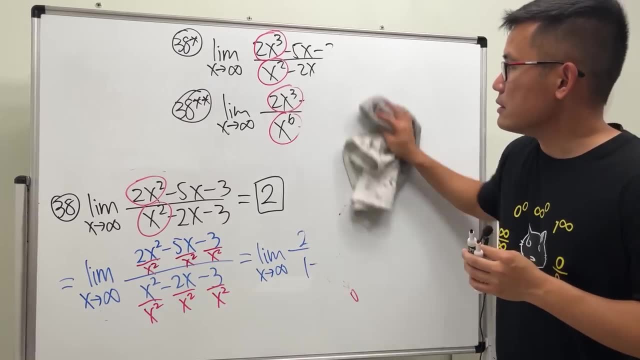 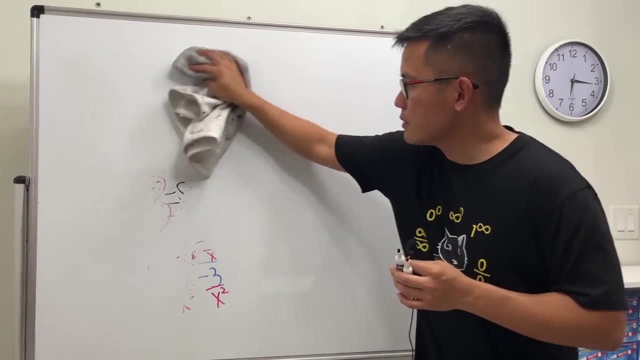 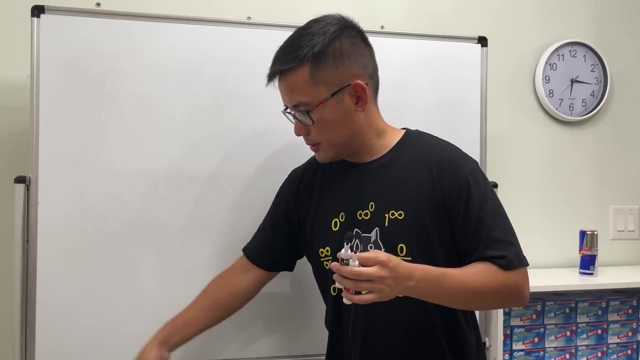 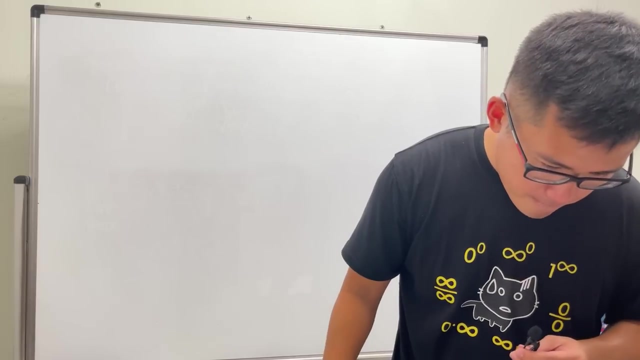 here is bigger, then you get zero. that's it. these are the limit questions that you do not want to miss on your calculus test. Thank you for watching this video. See you in the next one. Bye, bye. Alright, so that was 38, now let's look at 39.. 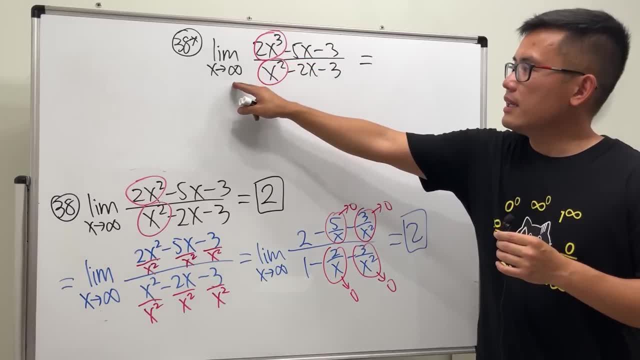 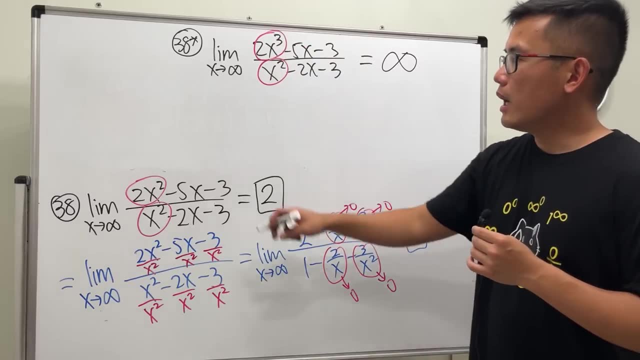 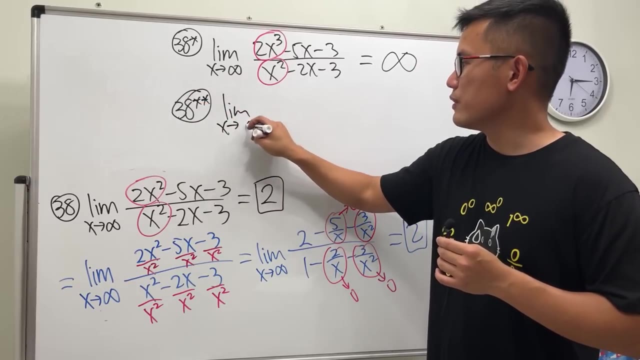 If you reduce, you just have x, As x goes to infinity. this right here will go to infinity. If the degree on the top is bigger, the whole thing goes to infinity. However, number 38,, star, star, If we have the limit as x approaches infinity, 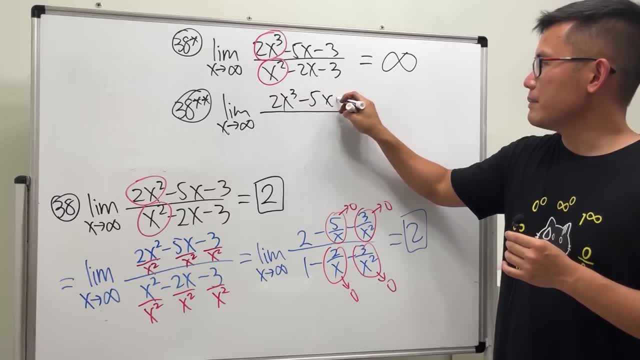 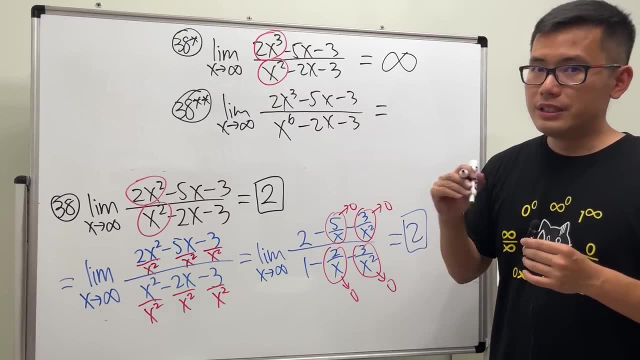 2x, let's say third power minus 5x, minus 3.. But if the bottom is x to the sixth power, and then minus 2x, minus 3.. You see, now the degree on the top is 3.. 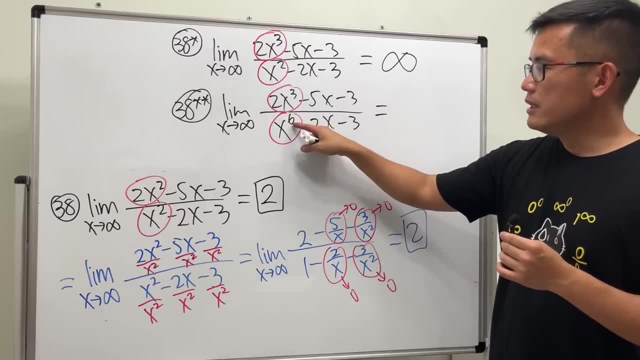 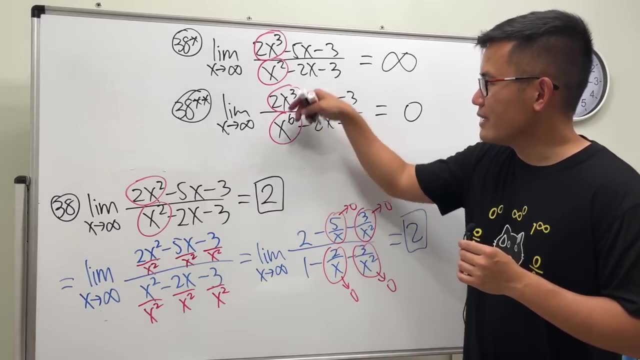 The degree on the bottom here is 3.. The degree on the bottom here is 6.. This is bigger than that. If the bottom is bigger, you get 0. Because you can reduce it right, You get 1 over x to the third power after you reduce. 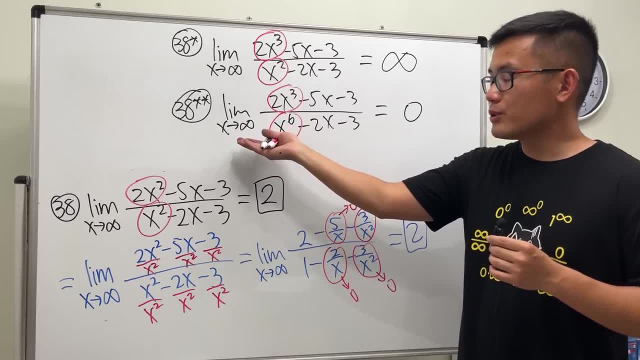 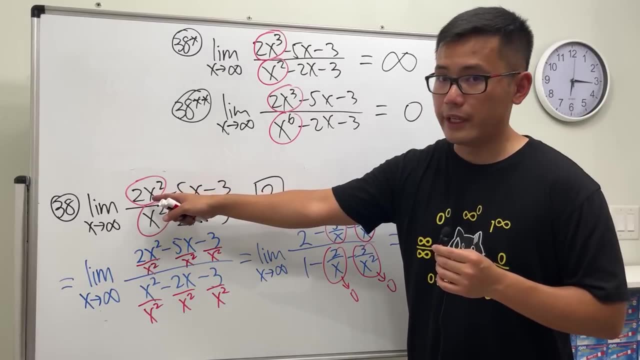 You have 2 over x to the third power. As x goes to infinity, you get 0.. So here are the three situations. You just compare the degree, aka the highest power of x on the top and also on the bottom. 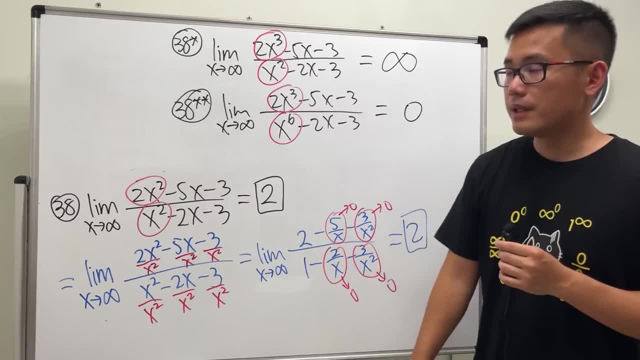 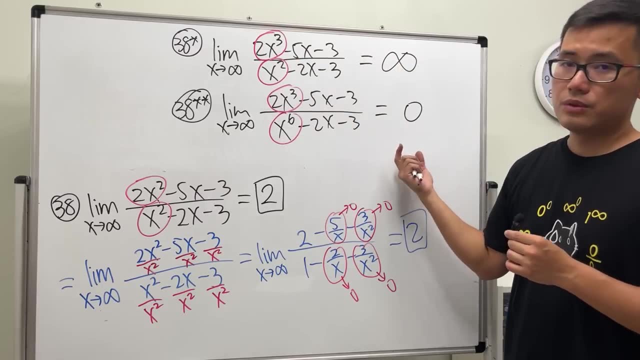 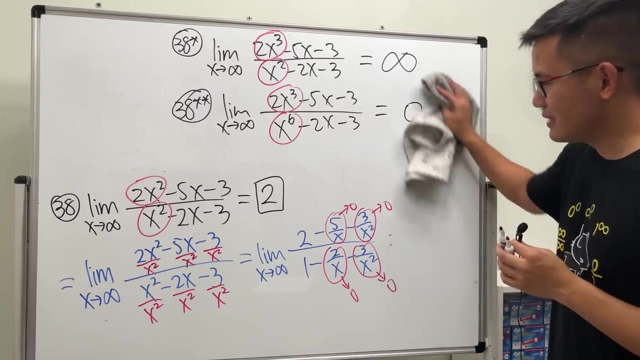 If they are the same, reduce the coefficient. If the top is bigger, then the answer will be infinity. If the bottom power right here is bigger, then you get 0. That's it. These are the limit equations that you do not want to miss on your calculus test. 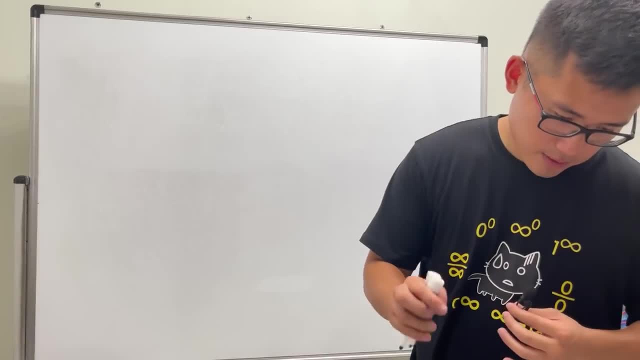 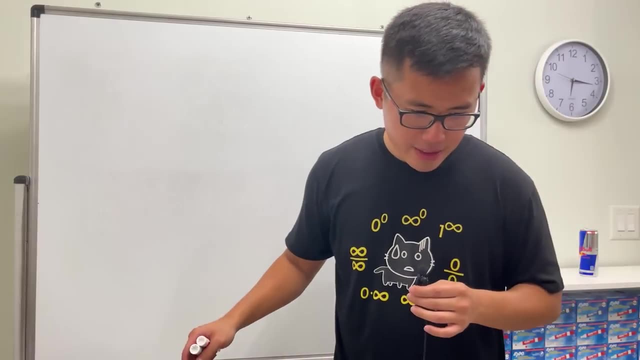 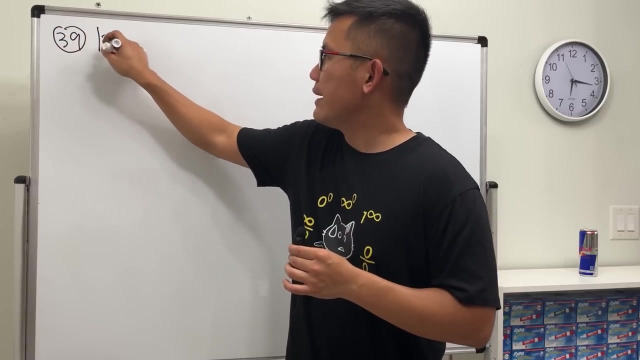 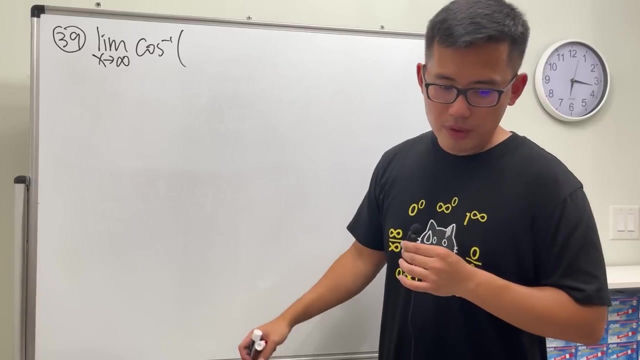 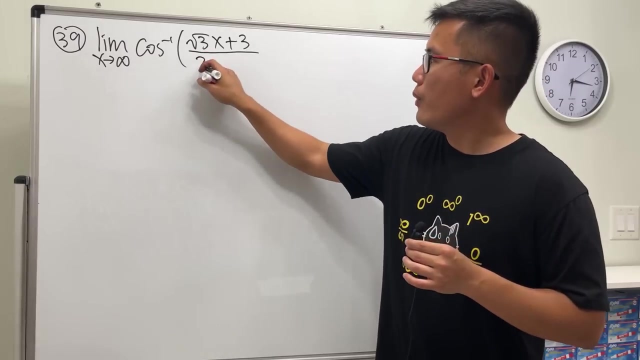 Alright, so that was 38.. Now let's look at 39.. Here we have the limit as x approaching infinity. We have inverse cosine, And then we have square root of 3.. x plus 3 over 2 over x minus 9.. 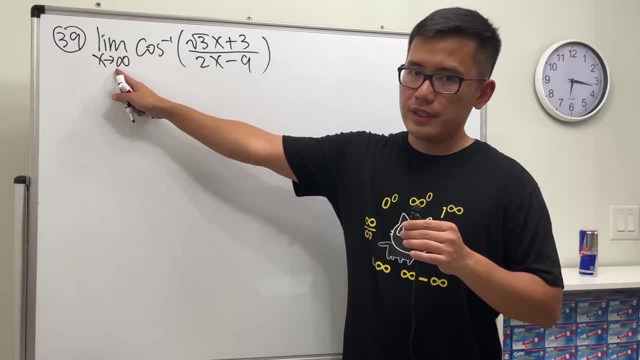 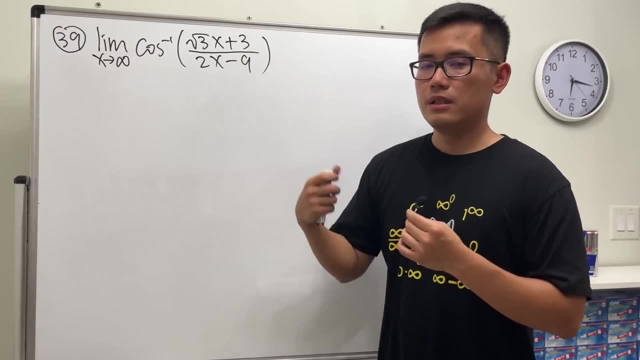 So let's do this the steady, fast, way. x is approaching infinity. We can do this inside out, So just look at it inside first. So, because x is approaching infinity, that's exactly what we talked about earlier. So just look at this, because that's x to the first power. likewise, that 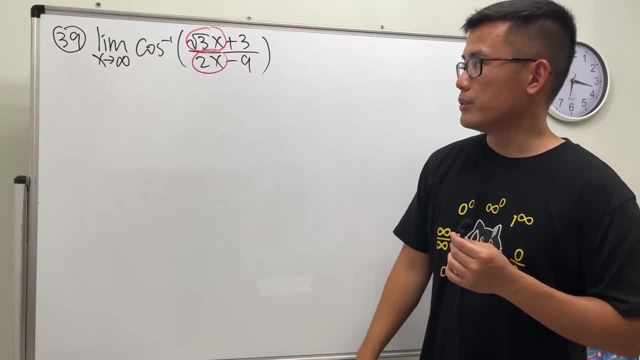 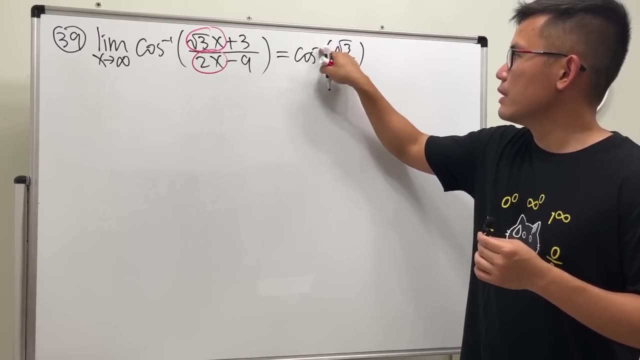 So in fact they cancel just square root of 3 over 2.. So this right here is just inverse cosine of square root of 3 over 2.. Now the hard question is: what's the inverse cosine of square root of 3 over 2?? 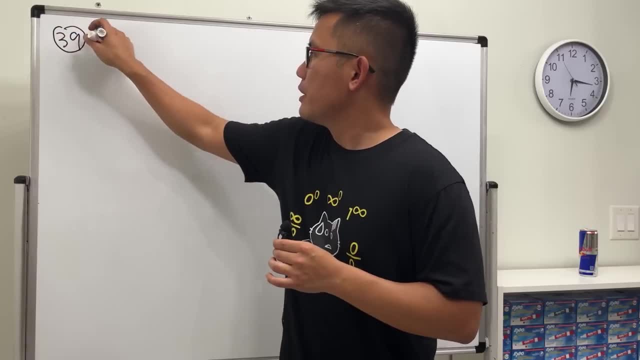 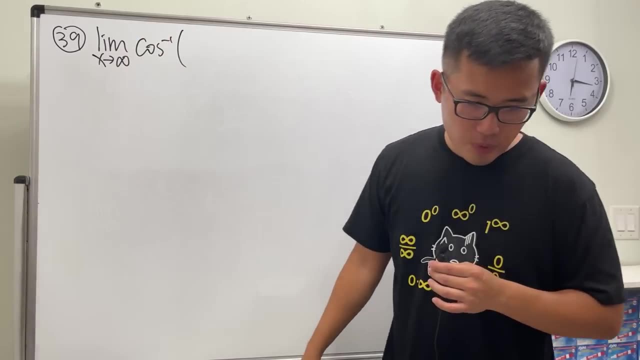 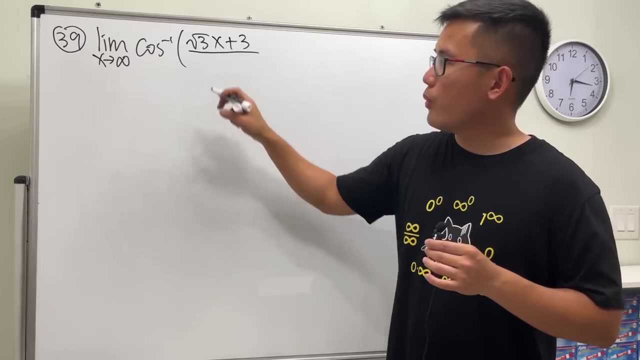 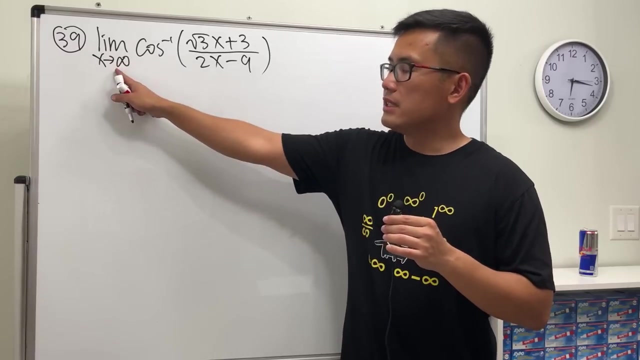 Here we have the limit as x approaching infinity. we have inverse cosine and then we have square root of 3, x plus 3, over 2x minus 9.. So let's do this the steady, fast way. x is approaching infinity. we can do this inside out, so just look at it inside first. 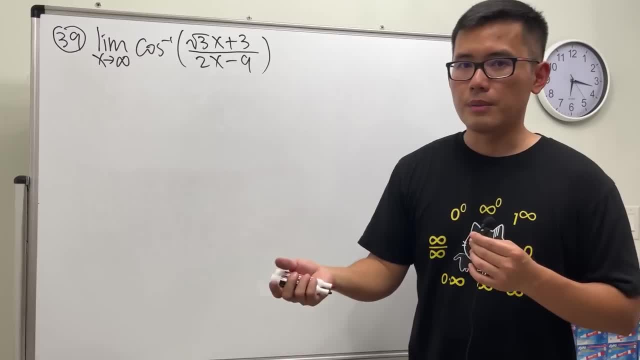 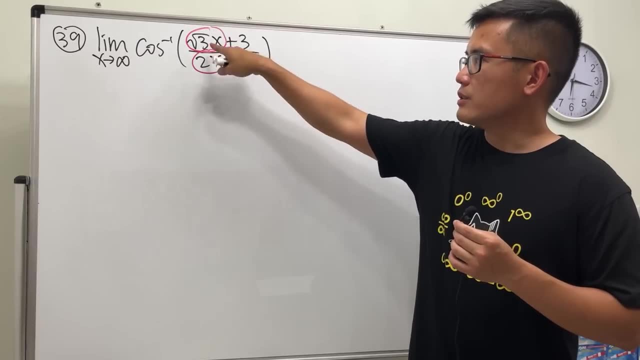 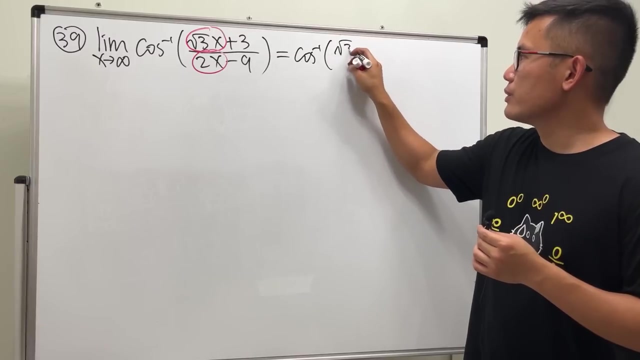 So because x is approaching infinity, that's exactly what we talked about earlier. So just look at this, because that's x to the first power, likewise that. So in fact they cancel just square root of 3 over 2.. So this right here is just inverse cosine of square root of 3 over 2.. 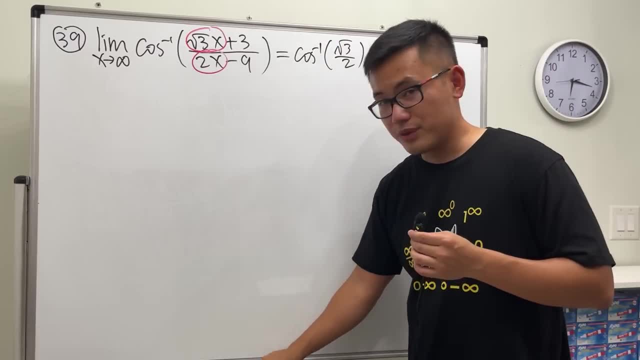 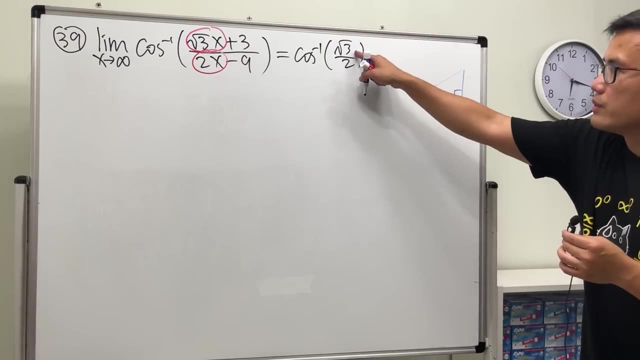 Now the hard question is: what's the inverse cosine of square root of 3 over 2?? Picture time: we have a right triangle, Square root of 3 is the adjacent and then the 2 is the hypotenuse, because we are talking about cosine, yeah. 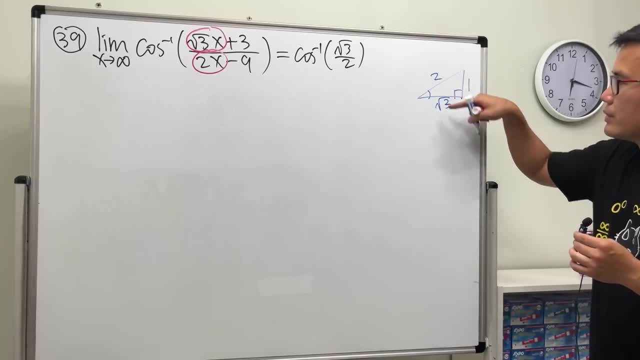 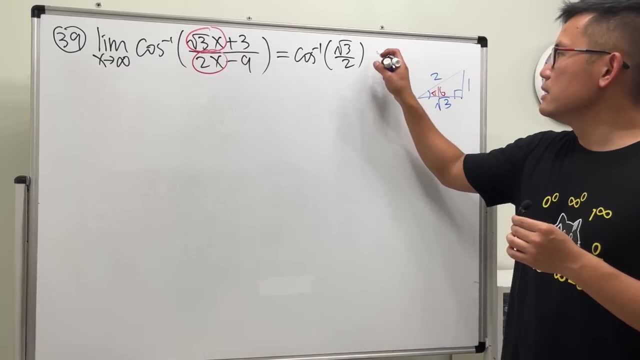 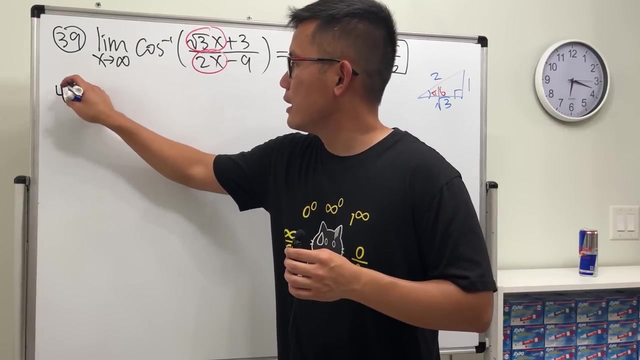 So this is the angle. it's again 1, 2, square root of 3, so this right here is pi over 6, 30 degrees. This is pi over 6, done, Alright, Alright, Alright, Alright. 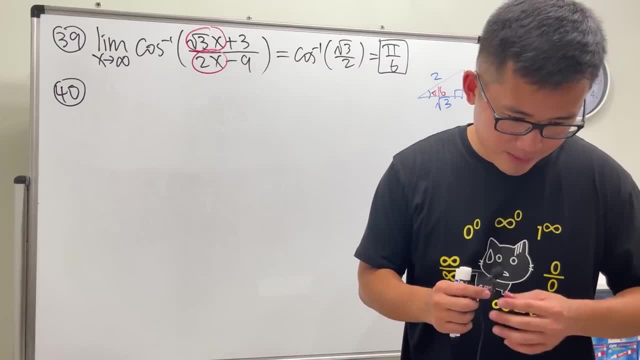 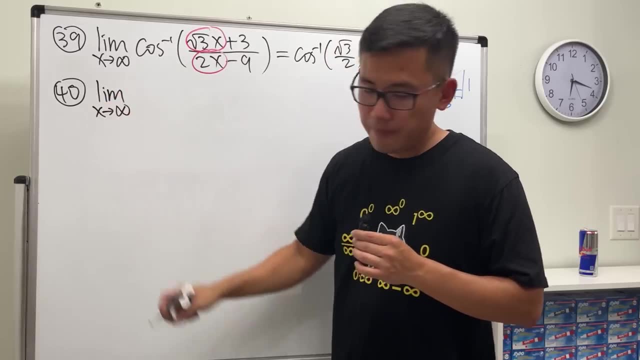 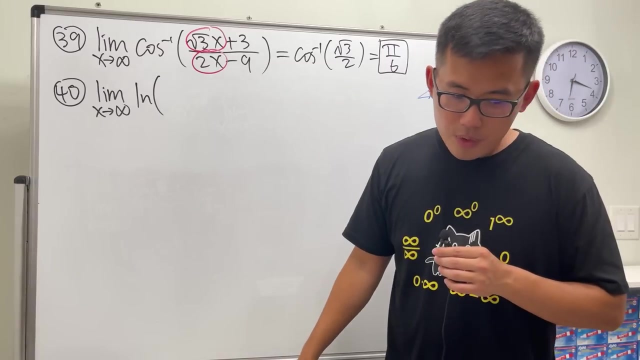 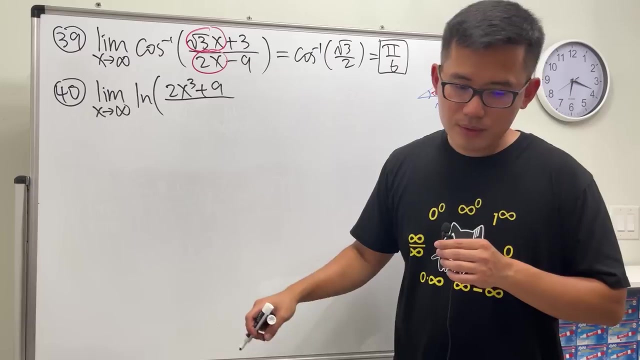 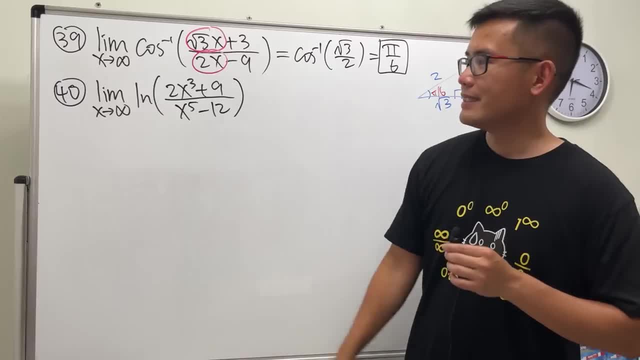 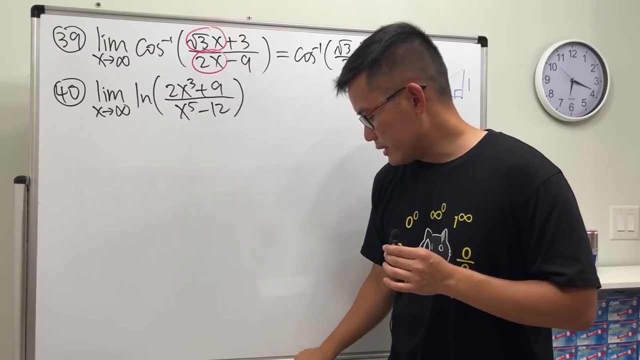 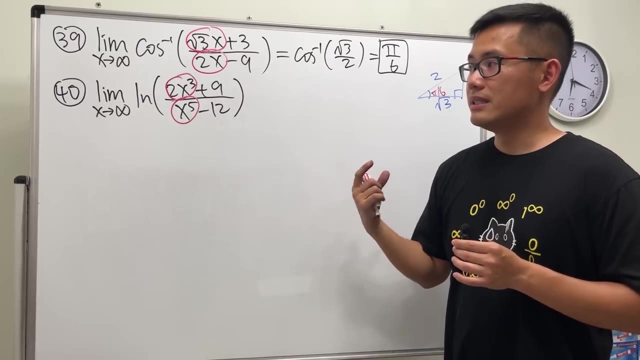 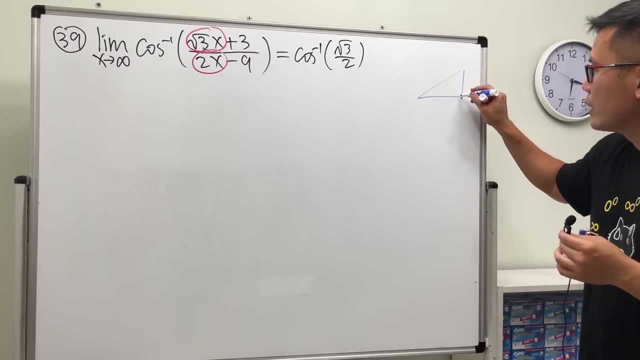 Picture time. We have a right triangle. Square root of 3 is adjacent And then the 2 is the hypotenuse, because we are talking about cosine. yeah, So this is the angle. It's again 1 to square root of 3.. 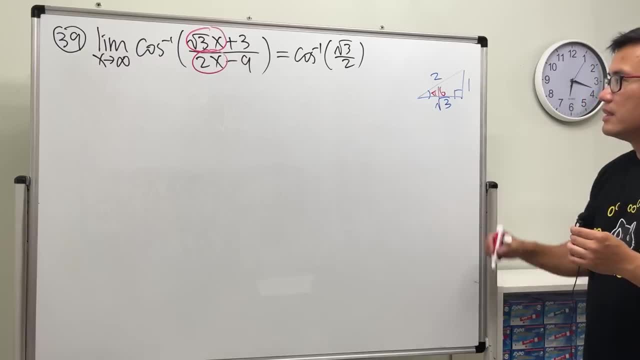 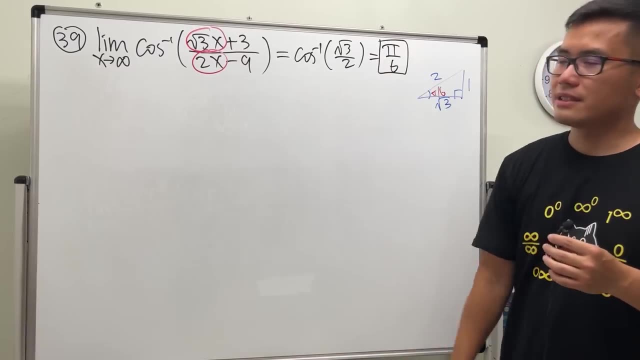 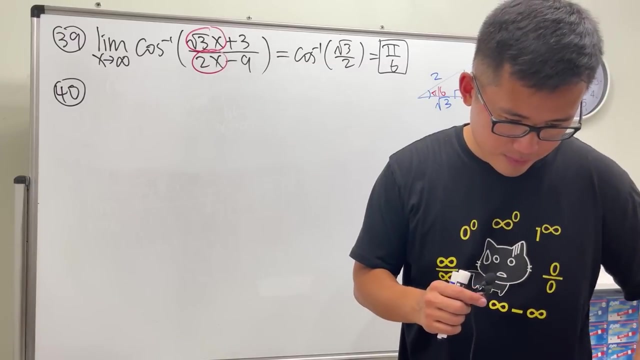 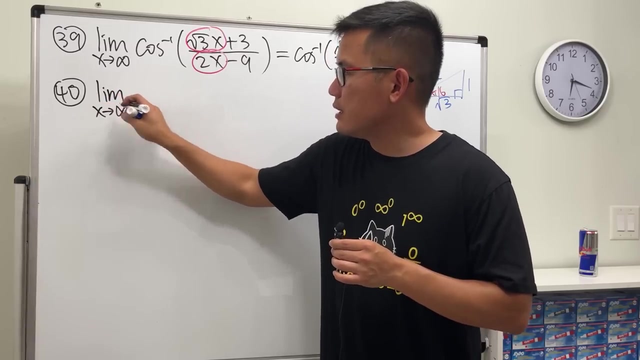 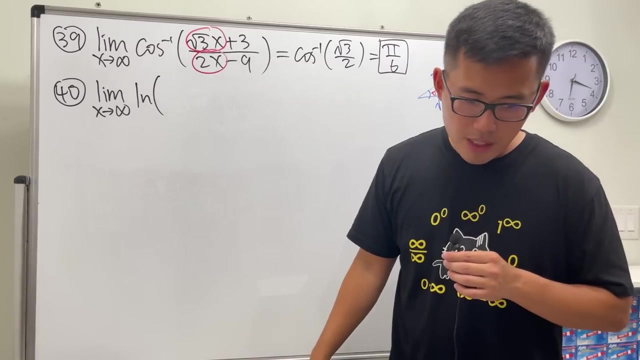 So this right here is pi over 6, 30 degrees, This is pi over 6.. Done Alright. next we have the limit as x approaching infinity, And then we have- let's do this- one ln of 2x to the third power plus 9.. 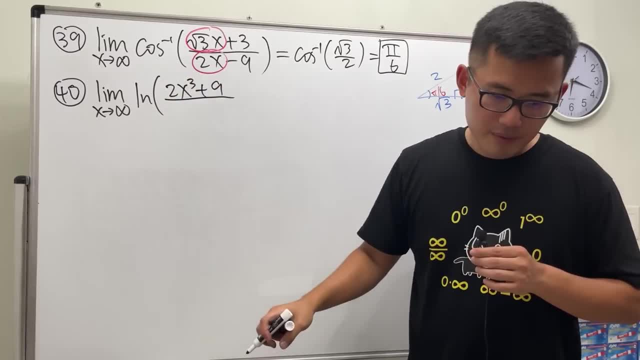 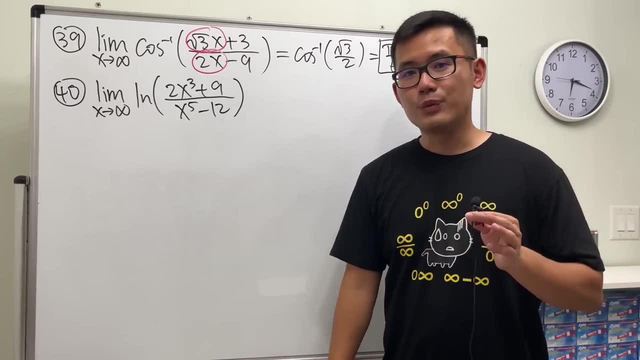 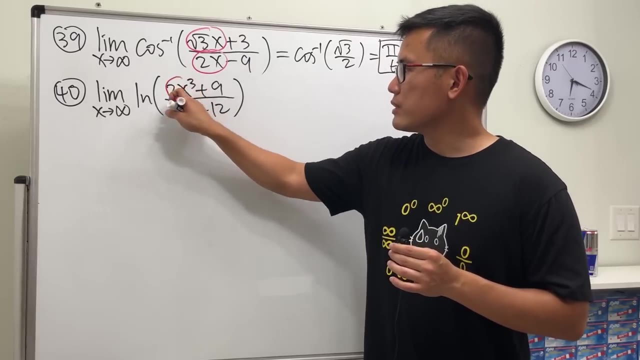 Over x to the fifth power minus 12.. Again, we can do this inside out, And this is x approaching infinity. So here let's just focus on 2x to the third power and then x to the fifth power. The degree on the bottom is bigger. 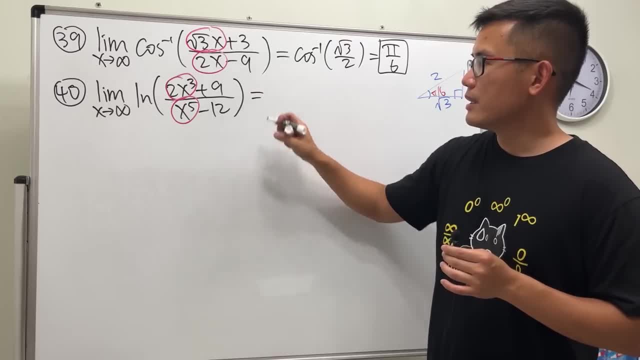 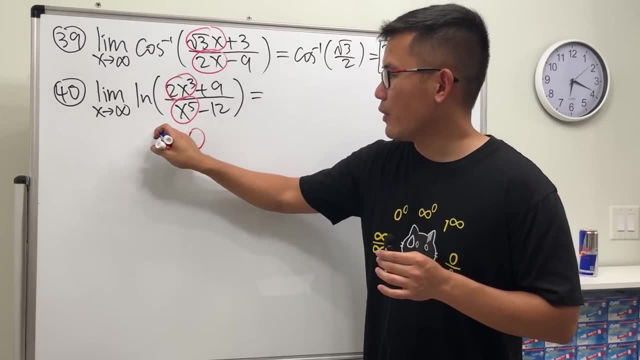 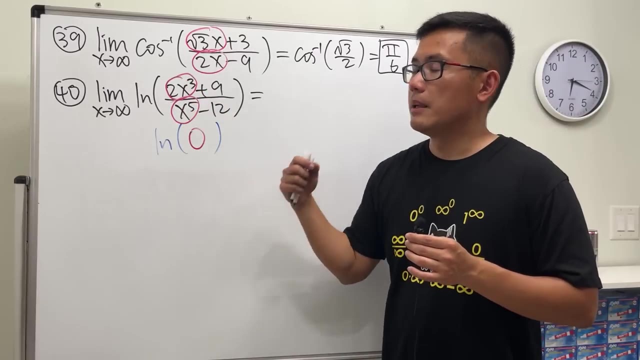 So we get 0.. So this right here is- I should write it down like this Marker here Inside: here we get 0, right, And then we have ln. But ln 0 is not really a thing, But technically this inside is positive. 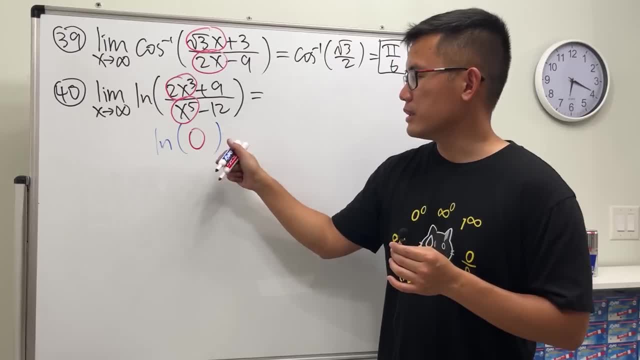 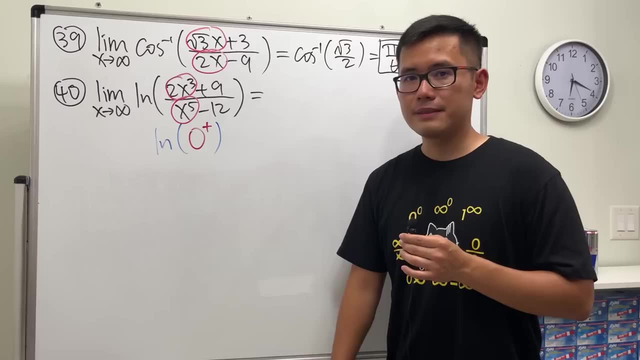 because when we have x approaching positive infinity, So this 0 is technically positive infinity. So what is ln of 0 plus? What did I say earlier? This is 0 plus. And then what's the ln of 0 plus? 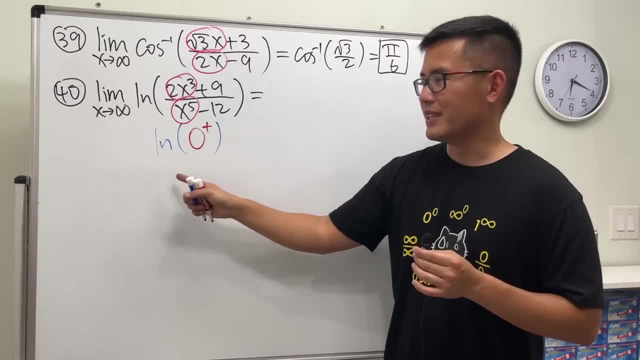 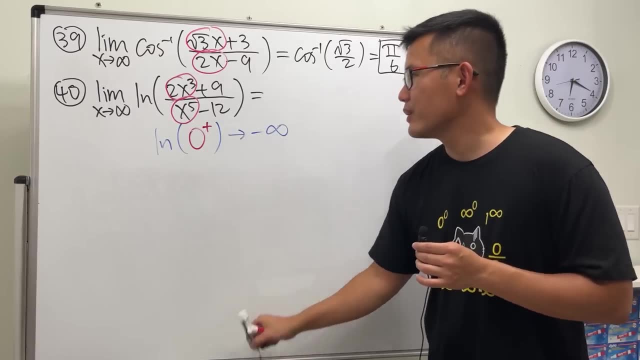 Yeah, there we go. This divided by that is 0 plus Sorry. And then what's ln of 0 plus Negative infinity Good. So yeah, you can just reason out this kind of questions in no time. That's why I said: 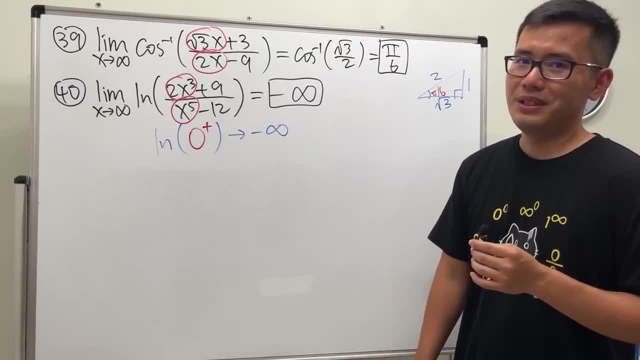 if you want to show work for this, it might be harder than it has to be. If you do this kind of things, I think we'll be happier. Usually, I like to ask this kind of questions in a multiple purchase format, So that way. 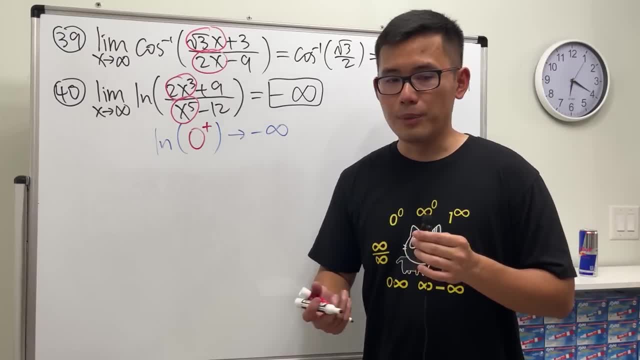 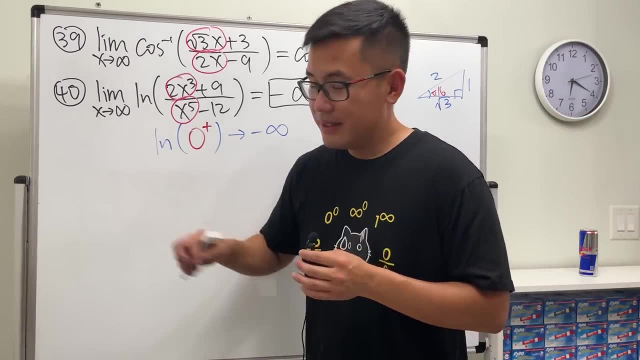 you guys don't have to struggle and you guys don't have to worry about how to show work. You just have to determine the answer. Yeah, I know it's just little thing, right, But my head, my arm, is still very tiring. 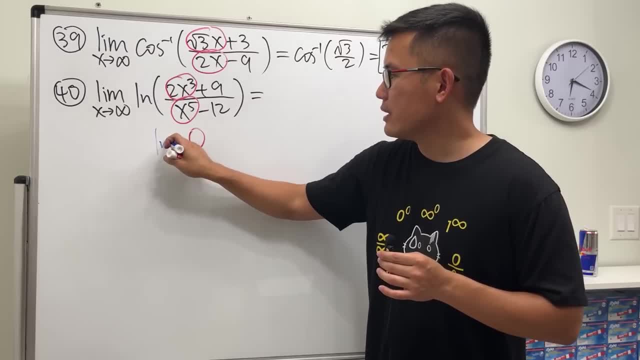 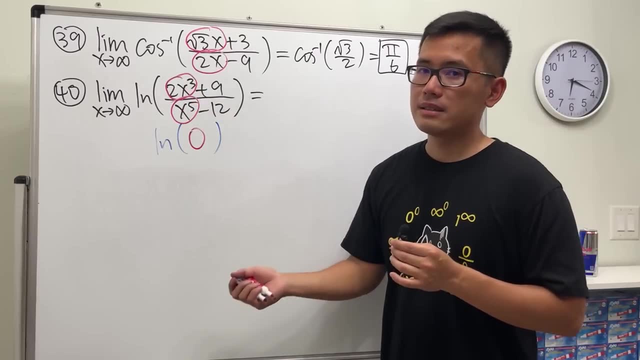 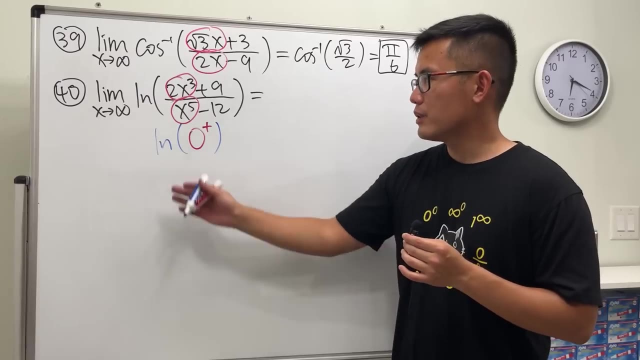 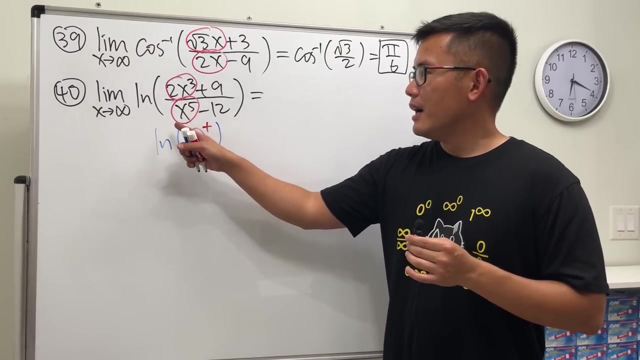 we get zero right, and then we have ln, but ln zero is not really a thing, but technically this inside is positive, because when we have x approaching positive infinity, so this zero is technically positive infinity. so what is ln of zero plus? what did i say earlier? this is zero plus. and then what's the ln of zero plus? yeah, there we go, this divided by that zero. 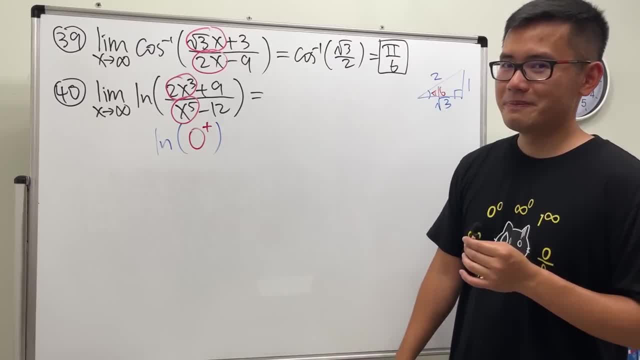 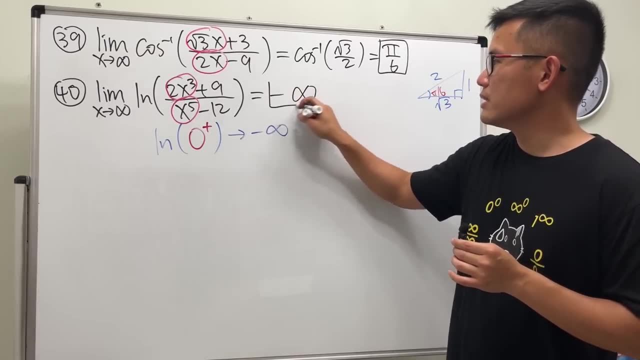 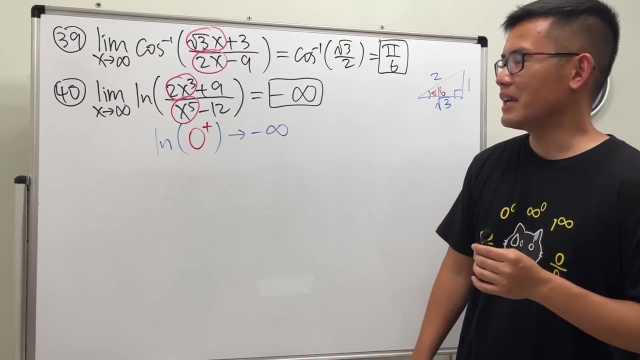 plus sorry, and then what's the ln of zero plus negative infinity? good, so yeah, you can just reason out this kind of questions in no time. that's why i said, if you want to show work for this, it might be harder than it has to be. if you do this kind of things, i think we'll be happier. 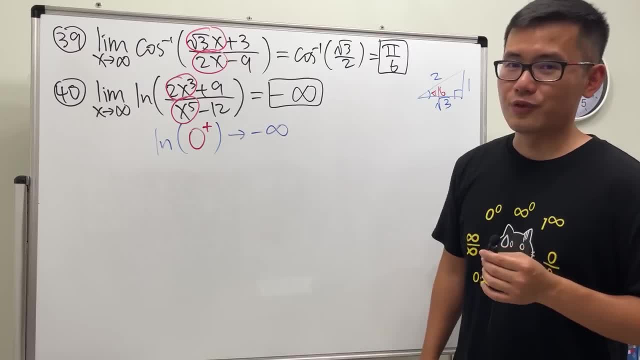 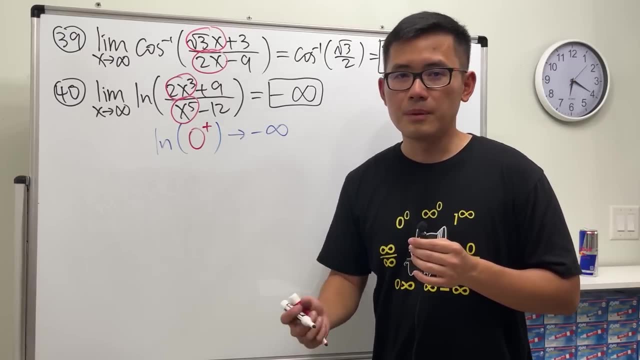 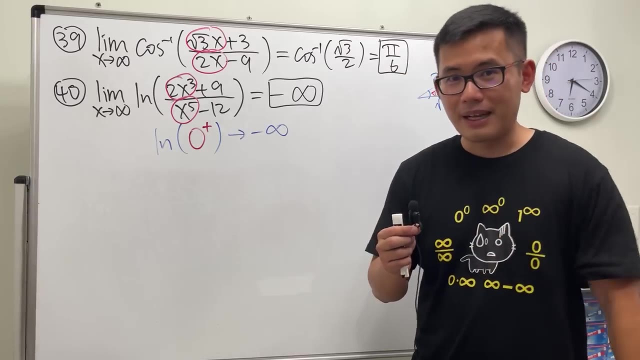 usually i like to ask this kind of questions in the multiple purchase format, so that way you guys don't have to struggle and guys don't have to worry about how to show work. you just have to determine the answer. yeah, i know, it's just little thing, right by my. 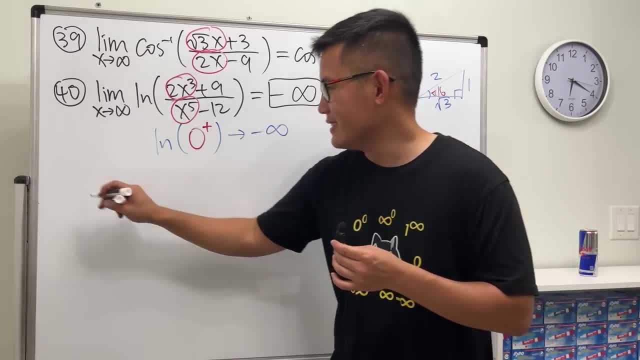 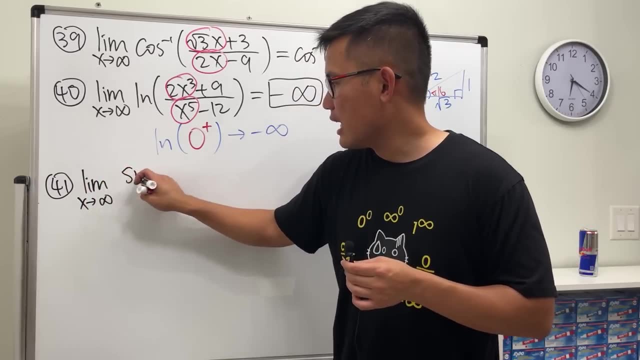 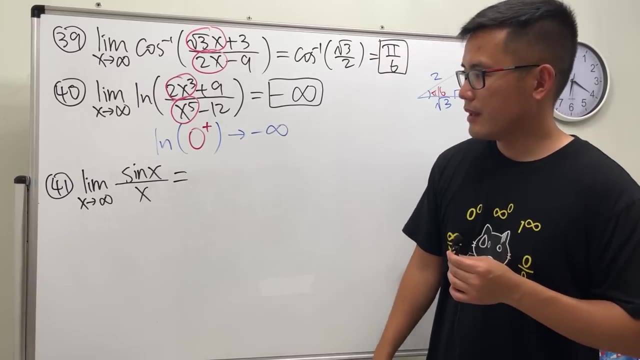 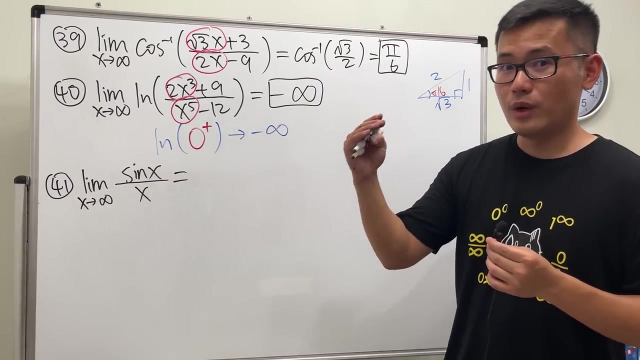 hand my own, it's still very tiring. 41: i have a look at the limit as x approaching infinity. sine of x over x: what's the answer for this? we did this for question number five. sine of x is in between of negative one and one is finite. 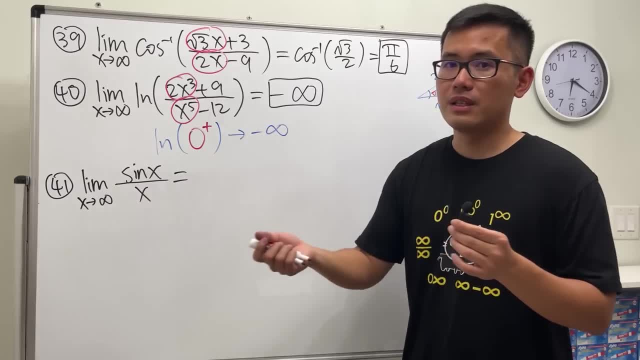 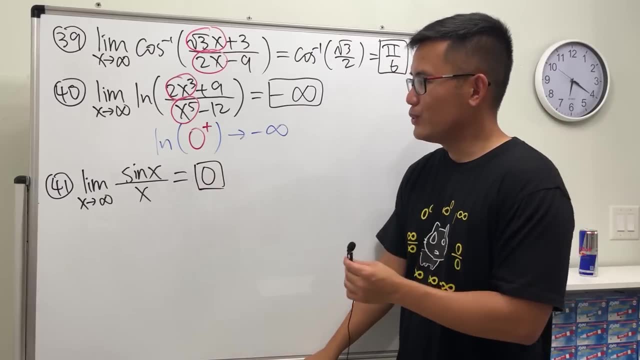 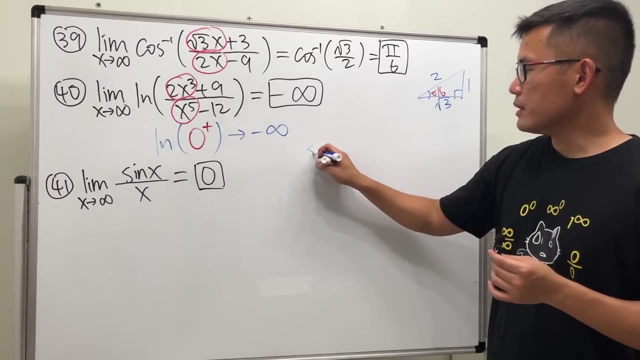 as x goes to infinity, the bottom is infinity. so you have a finite number divided by infinity. yeah, you get zero for sure. but if you want to do this a steady, more legitimate way, you do it. you do it like this: this is called the squeeze theorem. the idea is that 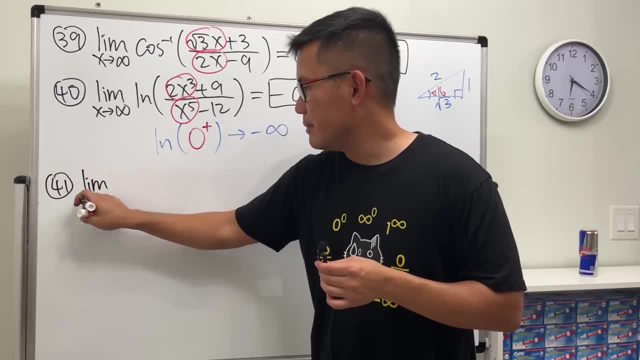 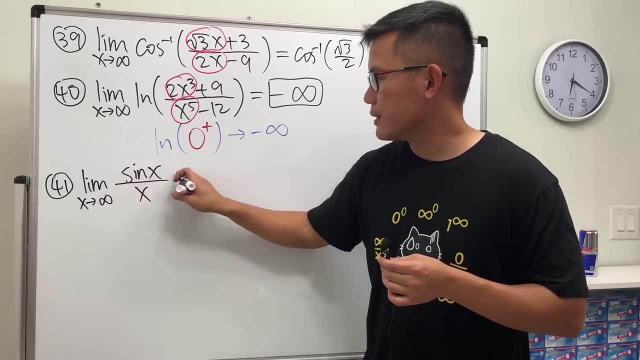 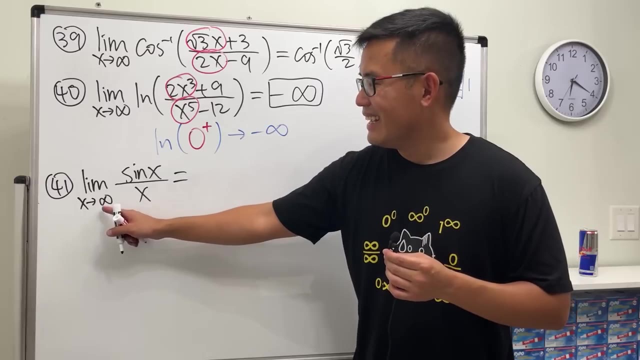 41. Have a look at the limit as x approaching infinity. sine of x over x. What's the answer for this? We did this for question number 5.. Sine of x is in between of negative 1 and 1. It's finite. 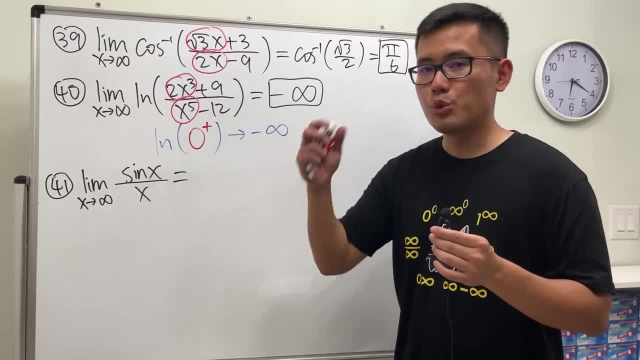 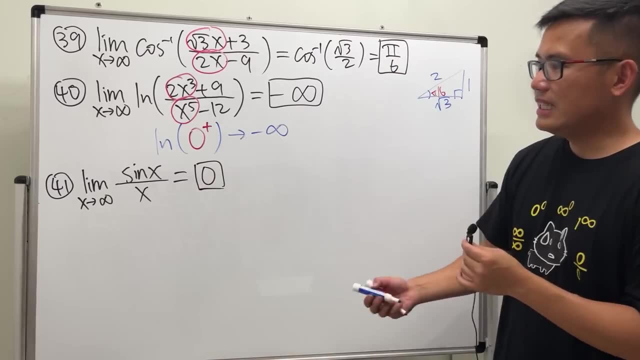 As x goes to infinity, the bottom is infinity. So if you have a finite number divided by infinity, yeah, you get 0. For sure. But if you want to do this a slightly more legitimate way, you do it like this: 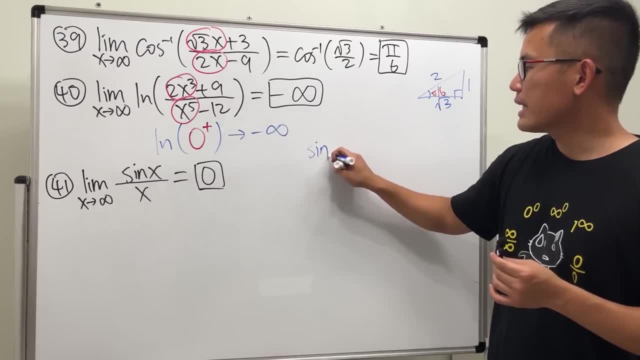 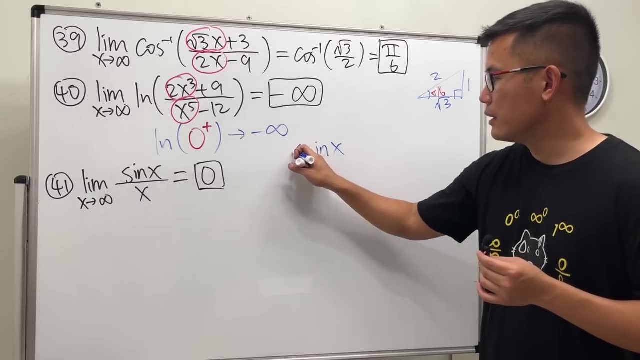 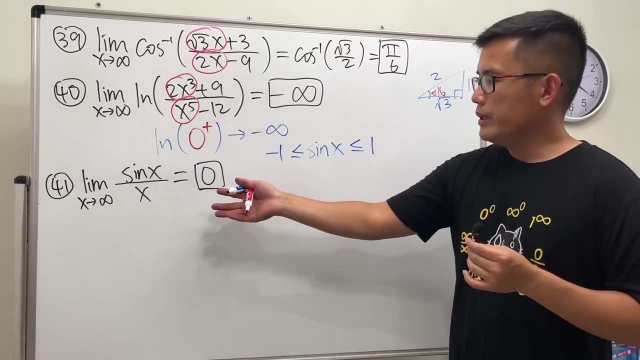 This is called the squeeze theorem. The idea is that you first have to mention that. okay, sine x is in between of negative 1 and 1.. So we can write this down: This is our inequality. Cool, And now we can divide everybody by x. 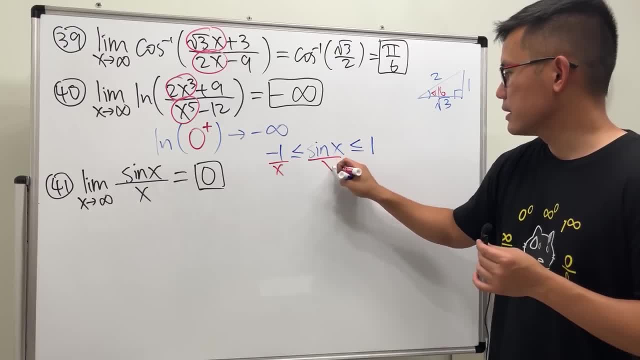 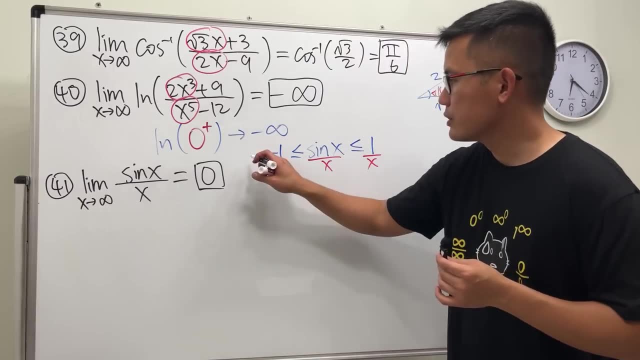 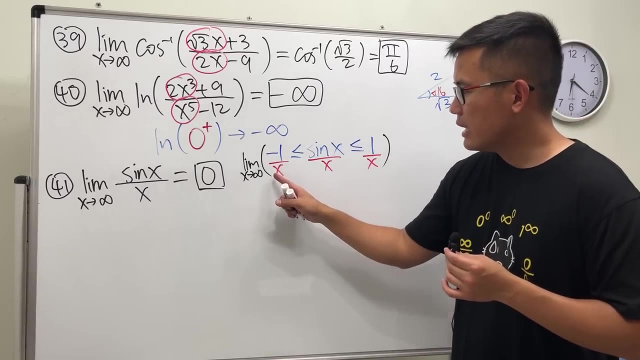 So that's what we are looking at, right? So divide everybody by x, Like so Good, And then we will take the limit as x goes to infinity for everybody. And if you do that, you can see that this is the thing. 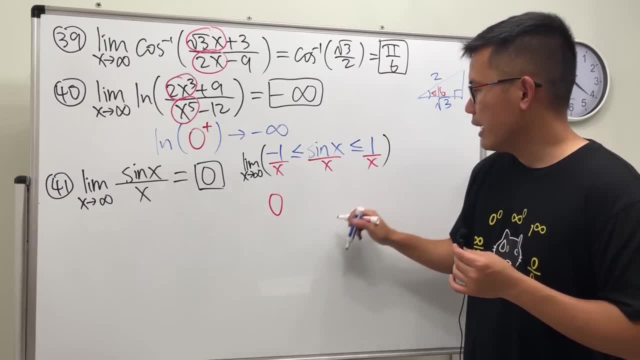 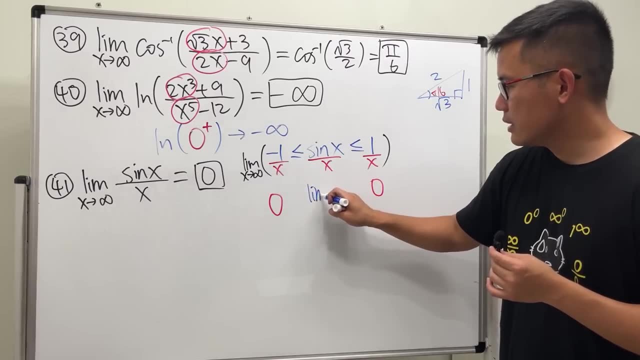 We have 0 here, And then 1 over x goes to infinity is also 0. And then in the middle is exactly what we are looking at: The limit as x approaches infinity, sine x over x, And as you can see, 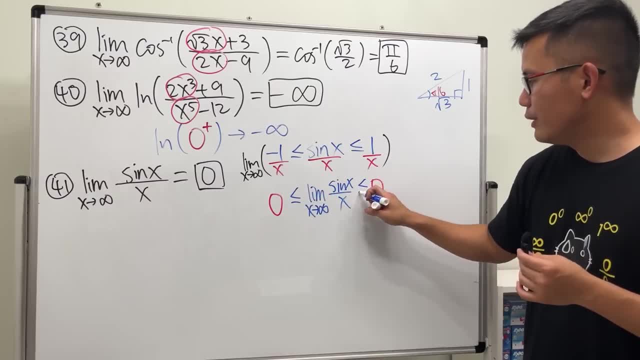 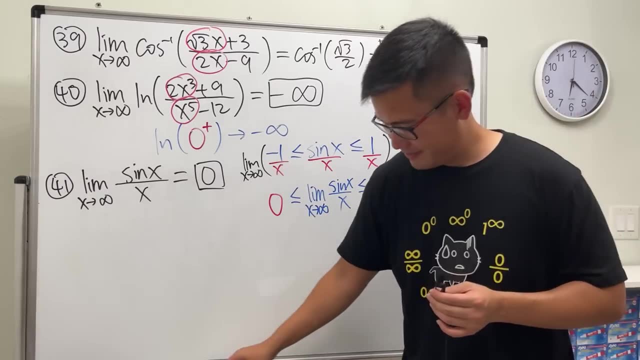 this limit is in between of 0 and 0.. Therefore, it has to be 0.. Done, It's a squeeze. It has to be 0.. Done, All right, Number 43.. I'm going to do 43,, 44,, 45.. 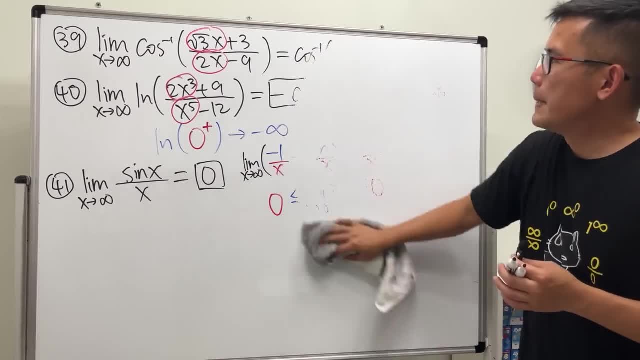 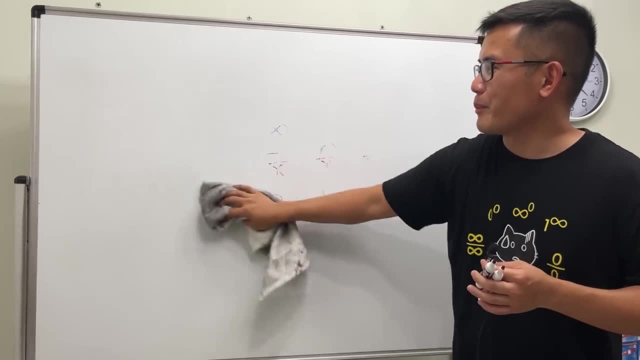 Hopefully Not possible. I don't think it's possible for me to do three questions on the same board. Maybe We'll try Number 43.. We have the limit as x approaches infinity, And then we have 0. And then 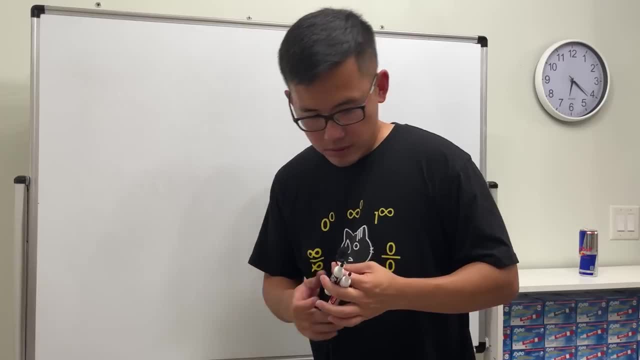 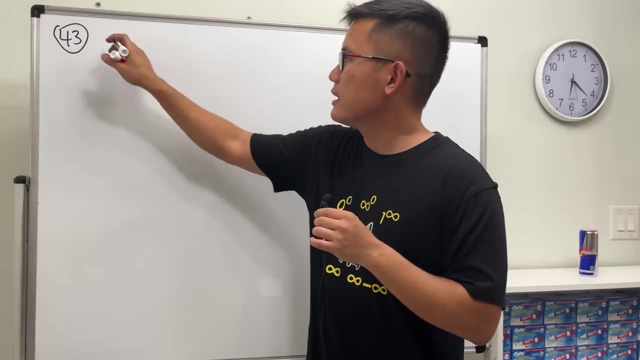 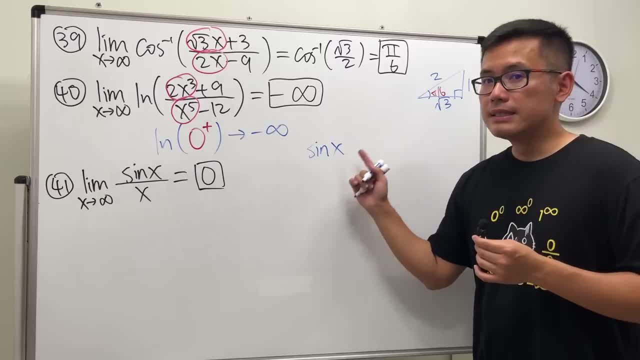 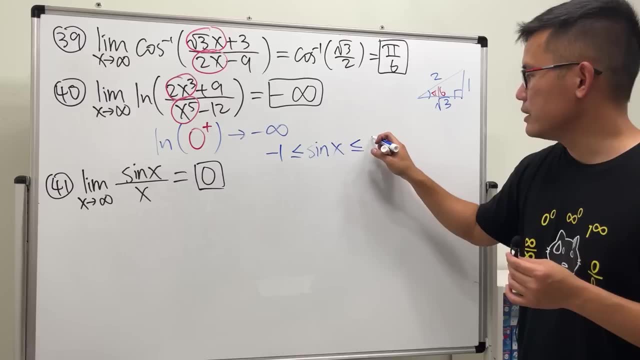 you first have to mention that. okay, sine x is in between of negative one and one, so we can write this down. and this is our inequality, cool. and now we can divide everybody by x. so that's what we can do. and now we can divide everybody by x. so that's what we can do. 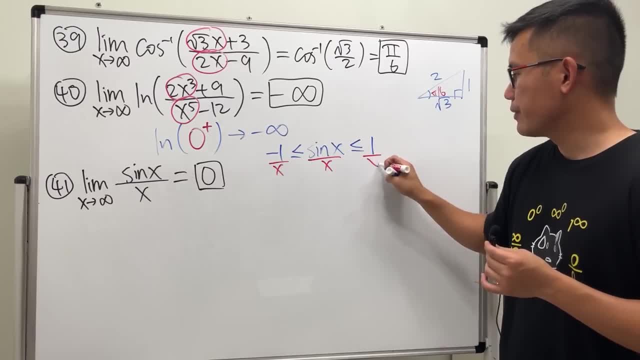 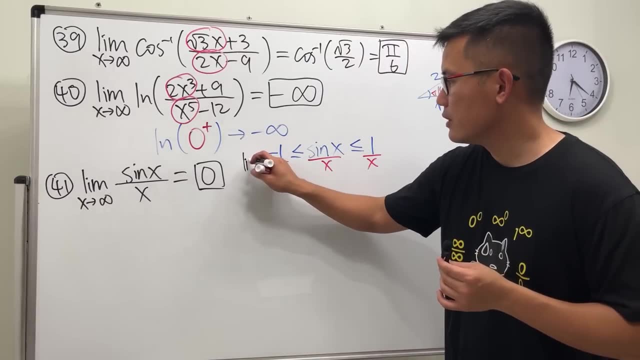 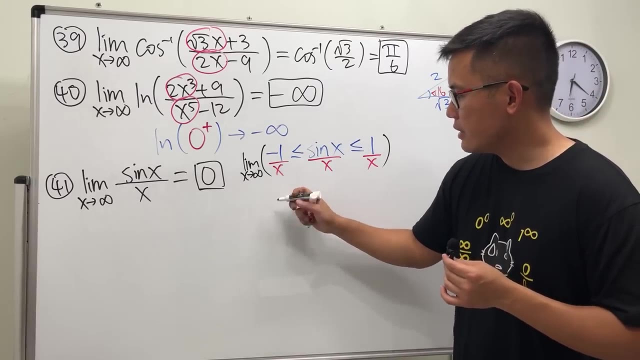 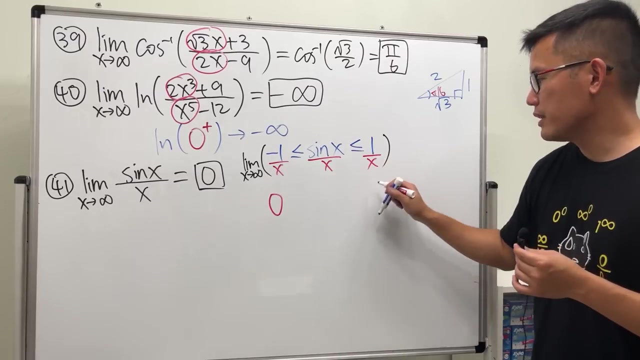 are looking at right, so divide everybody by x, like so good, and then we will take the limit as x goes to infinity for everybody. and if you do that, you're going to see that this is the thing we have: 0 here, and then 1 over 1 over x. x goes to infinity is also 0, and then in the middle, 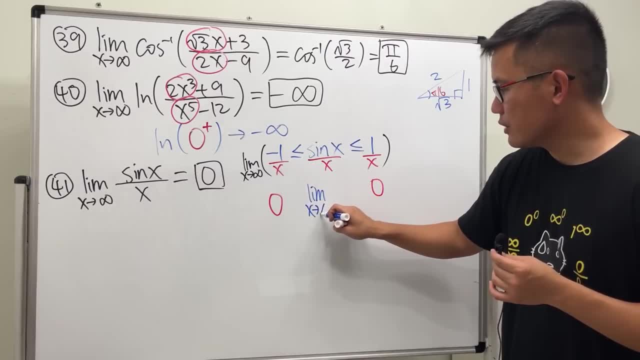 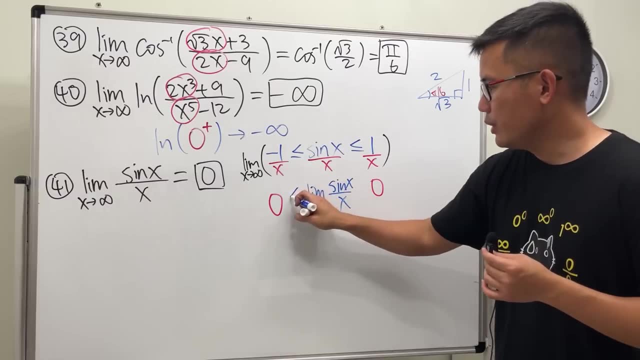 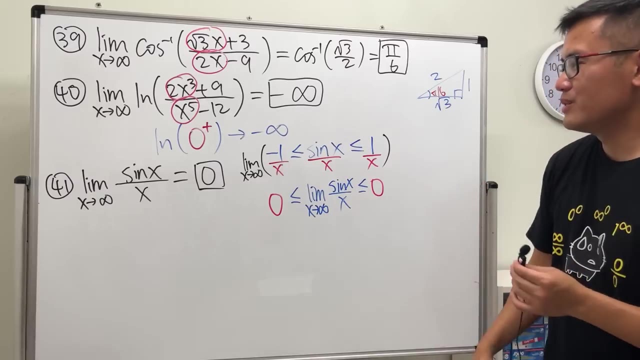 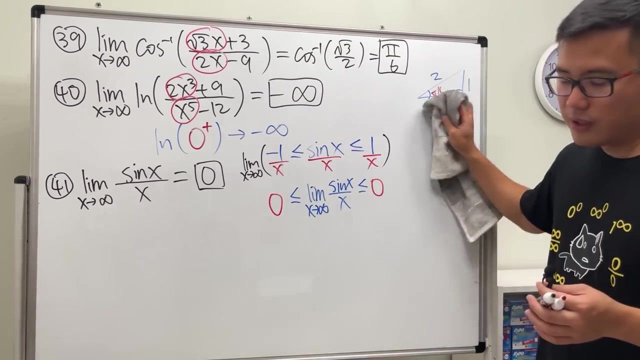 is exactly what we're looking at: the limit as x approaching infinity, sine x over x and, as you can see, this limit is in between of zero and zero. therefore, it has to be zero done, it's a squeeze. it has to be zero, done. all right, number 43. i'm going to do 43, 44, 45, hopefully. 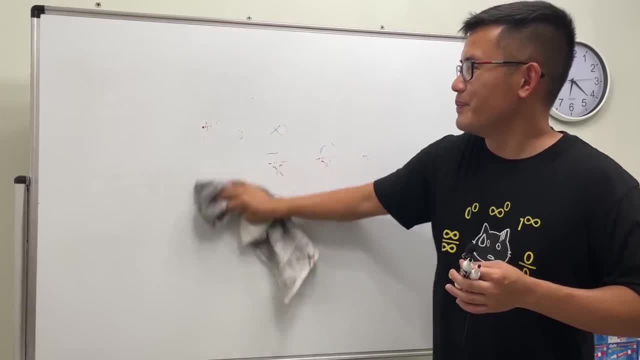 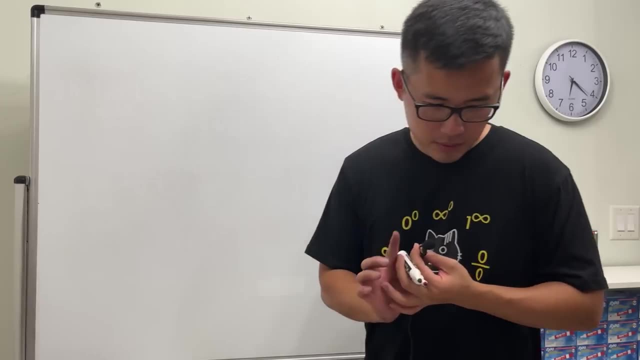 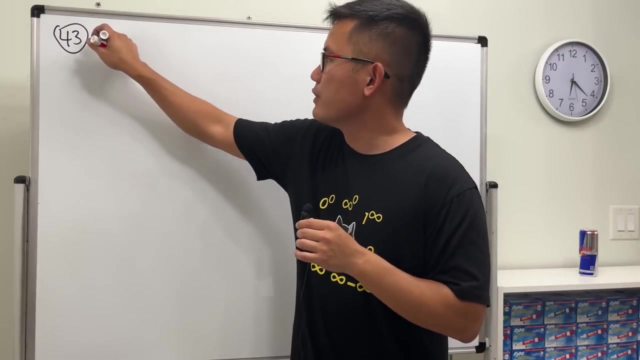 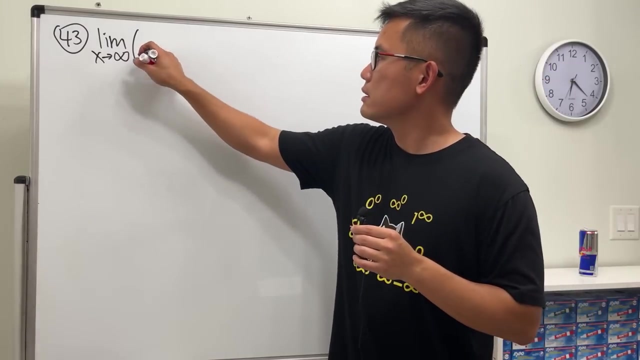 now not possible. i don't think it's possible for me to street questions on the same board. maybe we'll try number 43. we have the limit as x approaching infinity and we have square root of x plus 3 minus square root of x plus sorry. 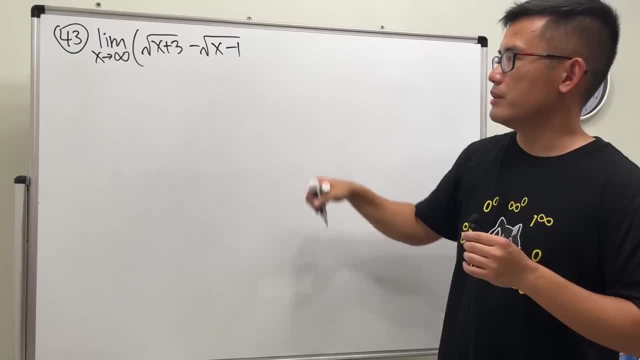 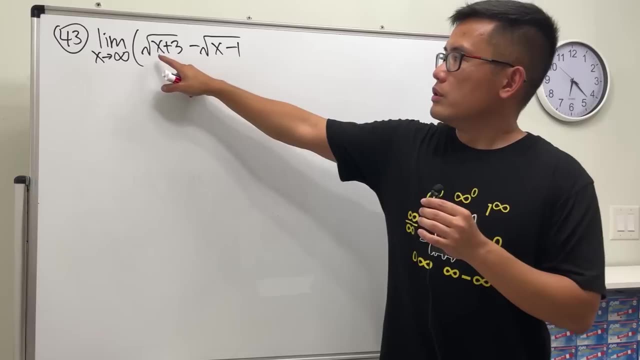 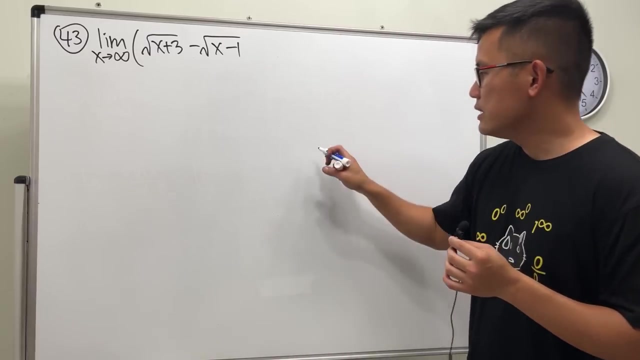 sorry, x minus 1.. i'm not going to close the parentheses for this one. let's see when we put infinity into here and here: square root of infinity plus you, just infinity. square root of infinity is infinity. and the reason is because if we have infinity for the base raised to a positive exponent, this right here will give us. 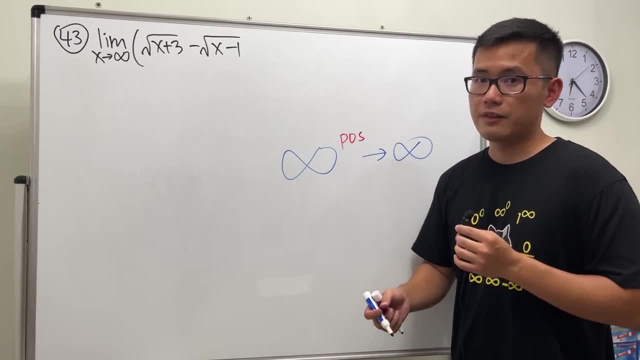 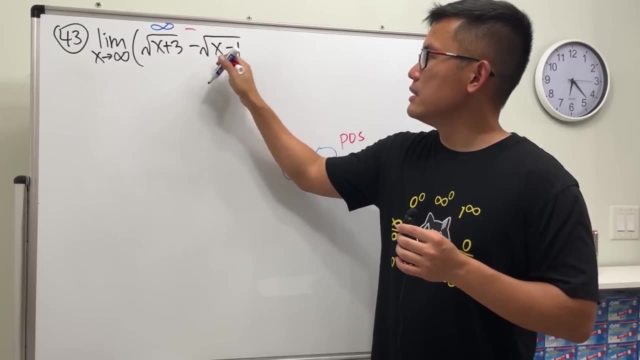 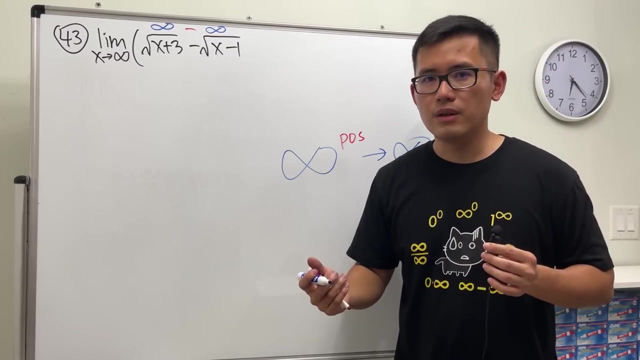 infinity and the square root is the same as saying one half power. so that's why square root of infinity gives us infinity and then minus- same idea, infinity. so we are talking about a new kind of indeterminate form for this video: infinity of infinity. the answer is not necessarily zero. why is infinity minus? 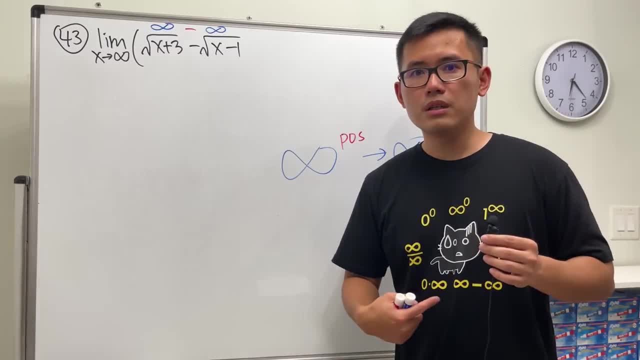 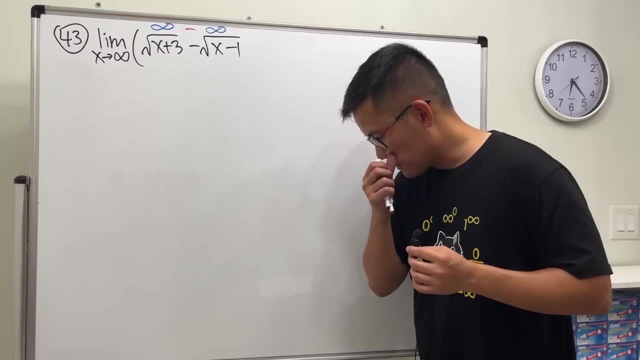 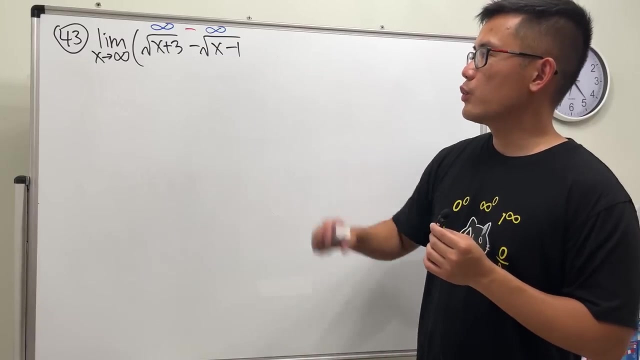 infinity in determinant form. it's right here. anything that you see right here is indeterminate, meaning that we cannot draw any conclusion yet. Well, how do we do it? Just like what we did before. when we see square roots: use the count you get and give. 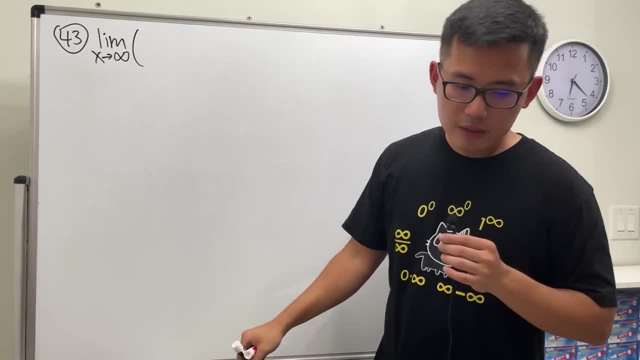 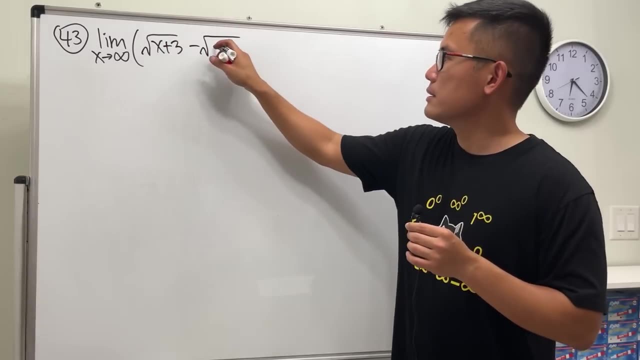 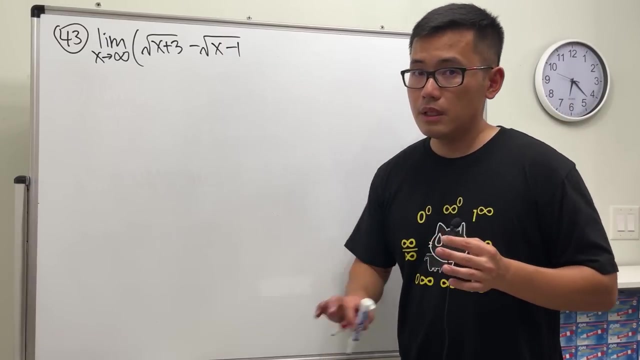 And, and we have a square root of x 1, 1, 1, times plus 3, minus square root of x plus times x minus 1.. I'm not going to close the parentheses For this one, for this one. 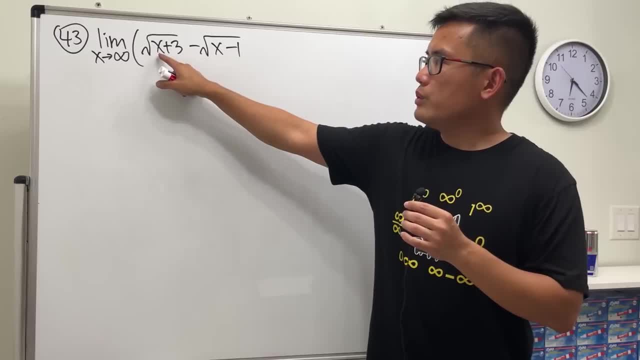 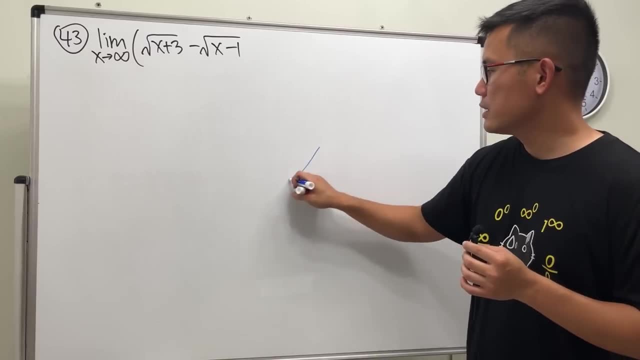 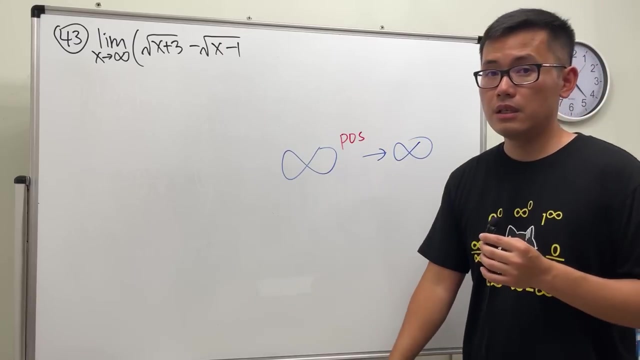 let's see When we put infinity into here and here, square root of infinity plus reduce to infinity, square root of infinity is infinity And the reason is because have infinity for the base raised to a positive exponent, this right here will give us infinity and the square root is the same as saying 1 half power. so 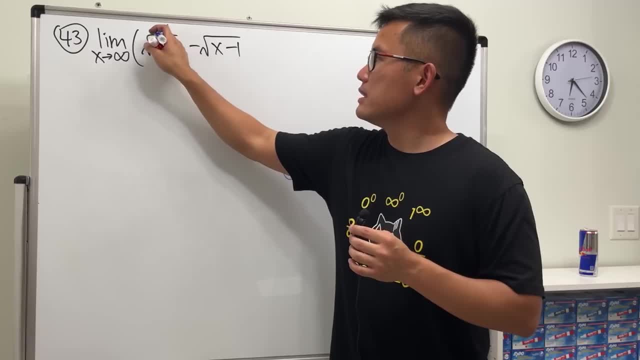 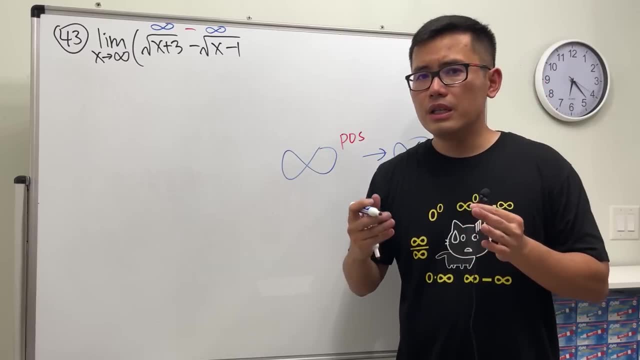 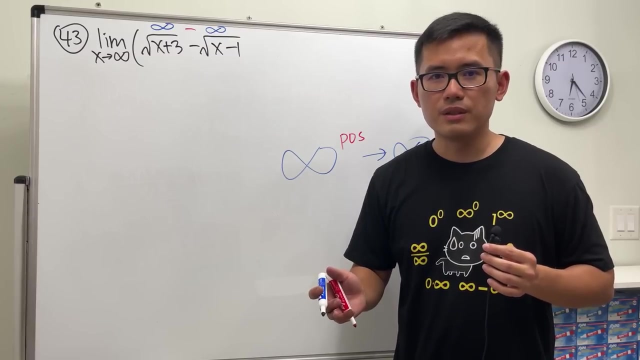 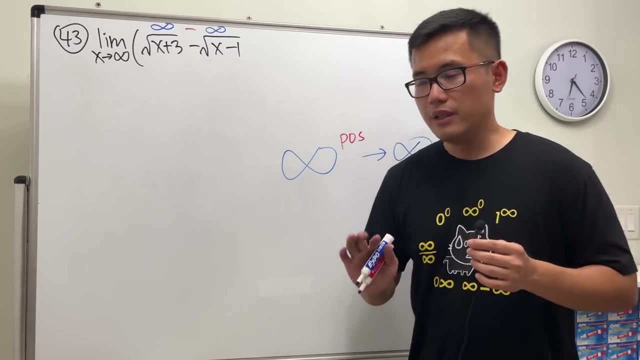 that's why square root of infinity gives us infinity and then minus. same idea. so we are talking about a new kind of indeterminate form for this video. infinity over infinity. the answer: it's not necessary: 0. why is infinity minus? infinity in the form? it's right here. anything that you see right here is. 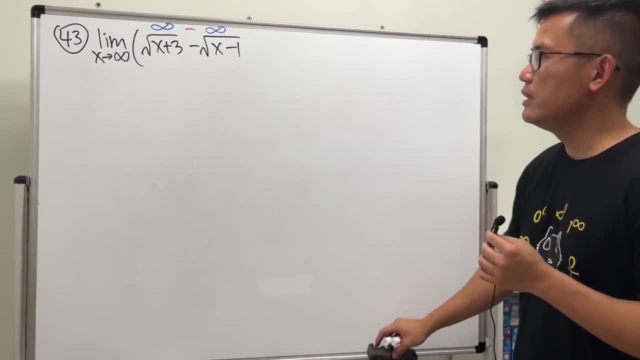 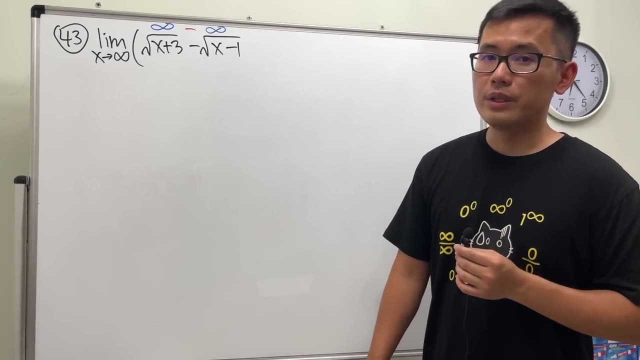 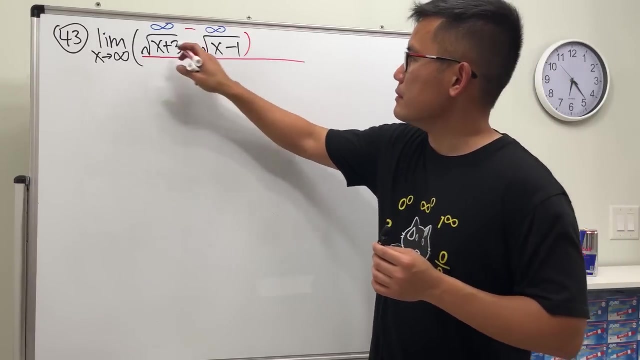 indeterminate, meaning that we cannot draw any conclusion yet. well, how do we do it? just like what we did before, when we see square roots, use the count you get and give it a try. let's multiply the top and bottom. that's why I didn't close. 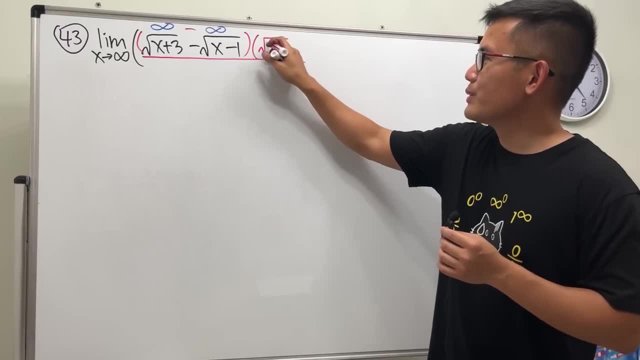 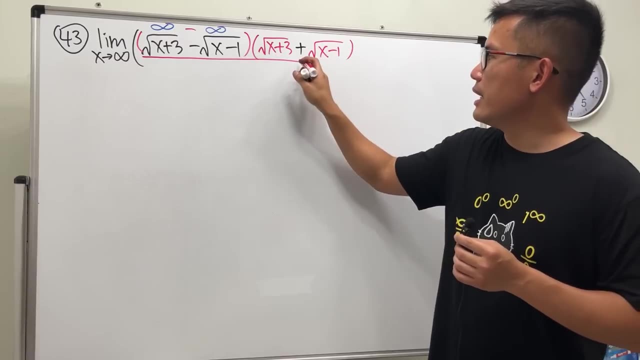 the parentheses. let's multiply the top of the pattern by square root of X plus 3, change this to a plus and the square root of X minus 1, and then let's do the same thing on the bottom: square root of X plus 3 plus square root of X plus 1. 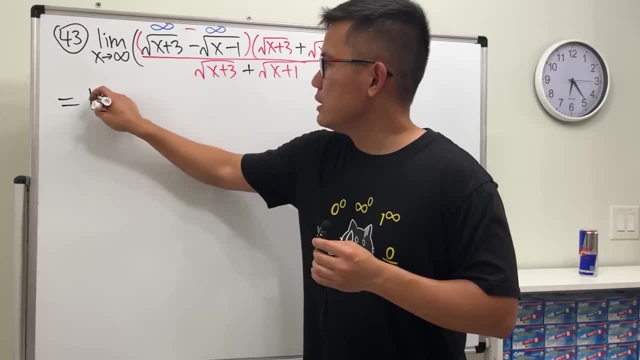 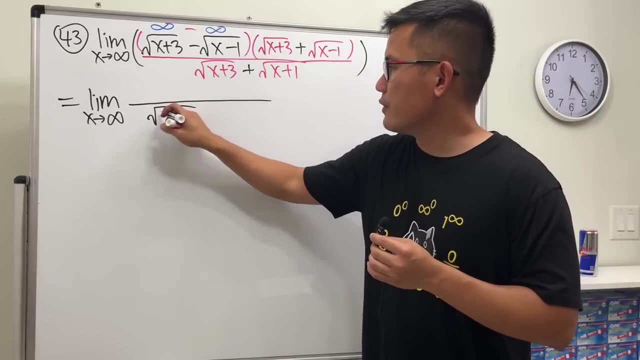 cool. now. this is the limit. as X approaching infinity, the bottom states the same: huh, so square root of X plus 3 plus square root of X plus 1. on the top, square root of X plus 3 plus square root of X plus 1, X minus 1, I put 2 characters. 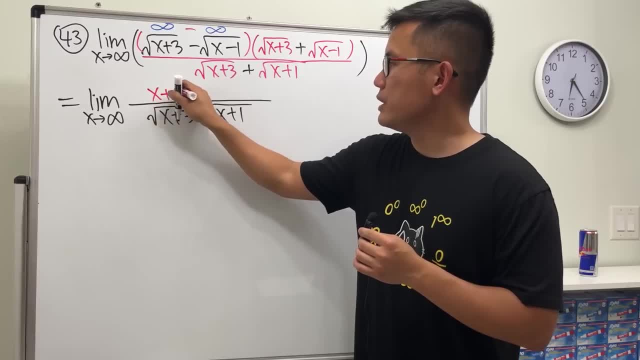 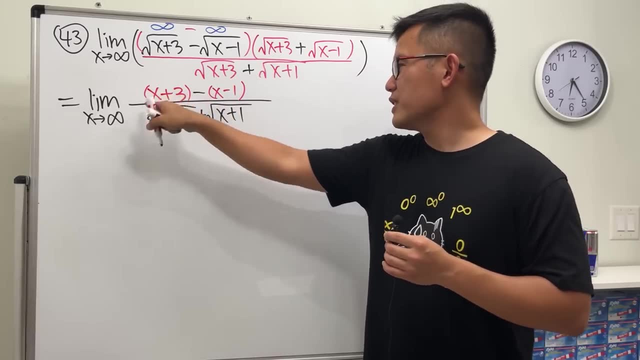 square root of Tabii, that's square root of X plus 1. on the top square root of X plus 3, Click on theORI, just go to first time, which is just x plus 3, and then minus square, the second square root of X plus 3, which is x minus 1, but you put permittees the first. 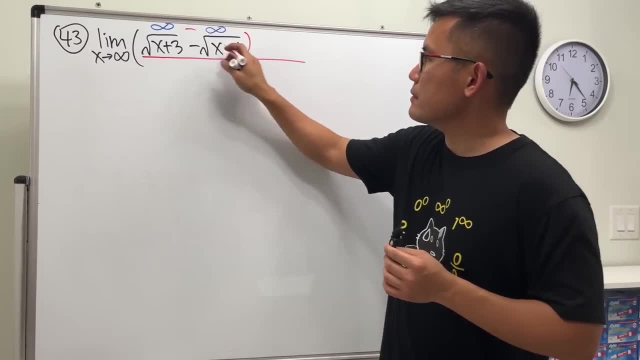 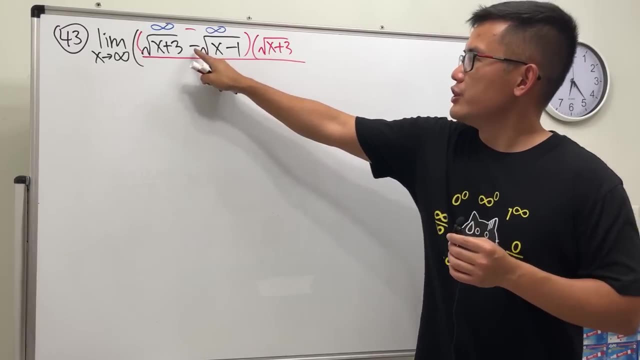 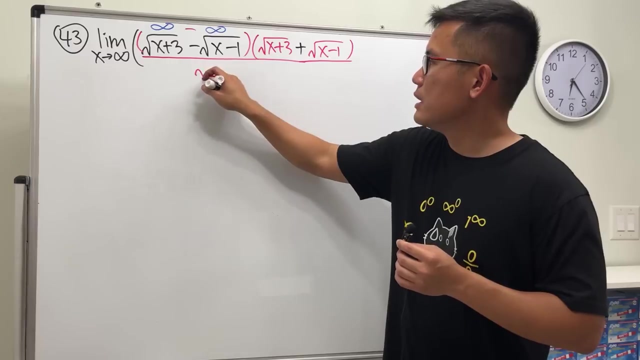 it a try. Let's multiply the top and bottom. that's why I didn't close the parentheses. Let's multiply the top and bottom by square root of x plus 3,, change this to a plus and a square root of x minus 1, and then let's do the same thing on the bottom. 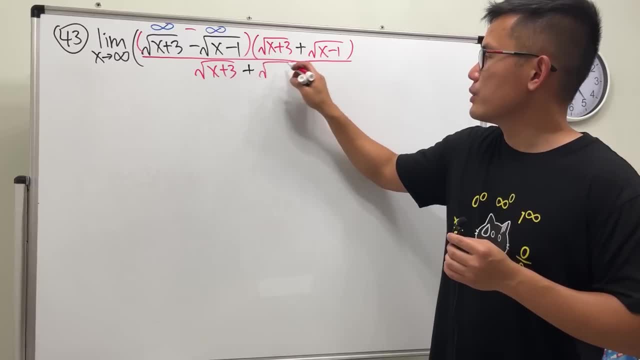 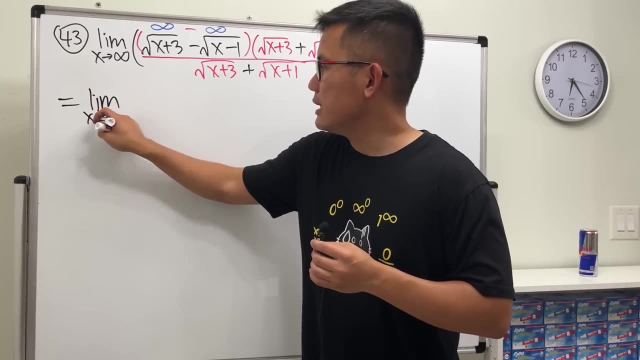 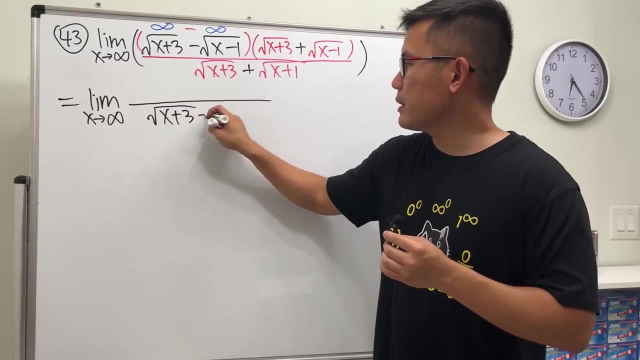 Square root of x plus 3 plus square root of x plus 1,. cool. Now this is the limit. as x approaching infinity, the bottom stays the same, huh, So square root of x plus 3 plus square root of x plus 1.. 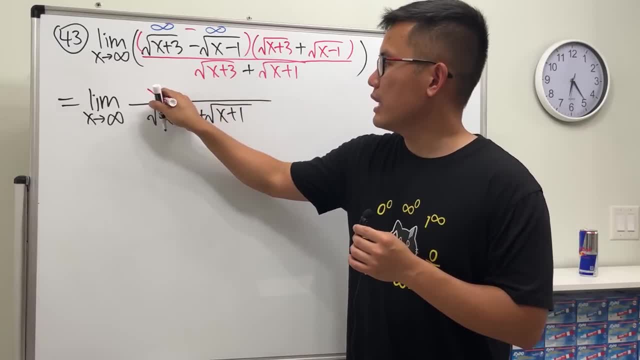 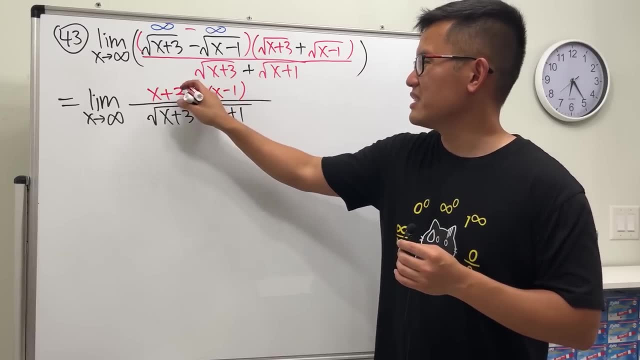 On the top. you just square the first term, which is just x plus 3, and then minus square the second term, which is minus square root of x plus 1.. So the answer is x minus 1, but you put parentheses. 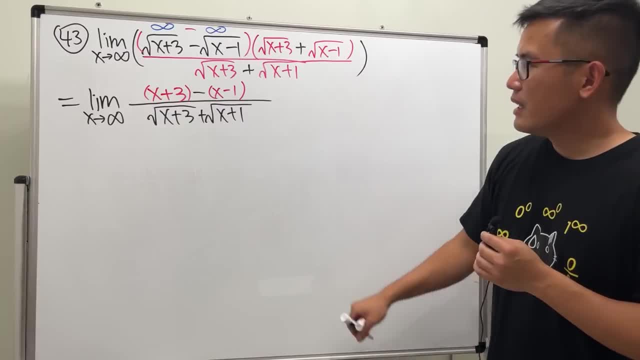 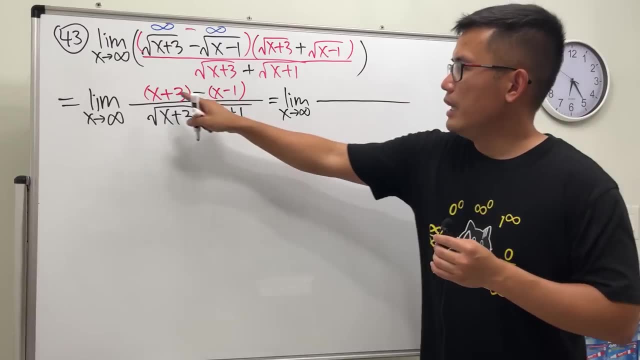 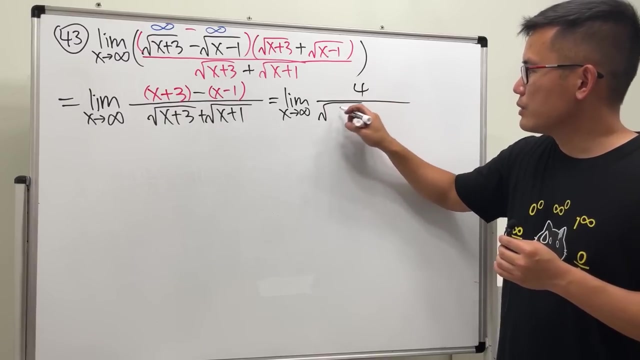 The first parentheses doesn't matter, but second parentheses does matter. Alright, and then we can simplify this. this is the limit as x approaching infinity, X minus x is gone, 3 minus minus, which is 4, so it's 4 over square root of x plus 3. 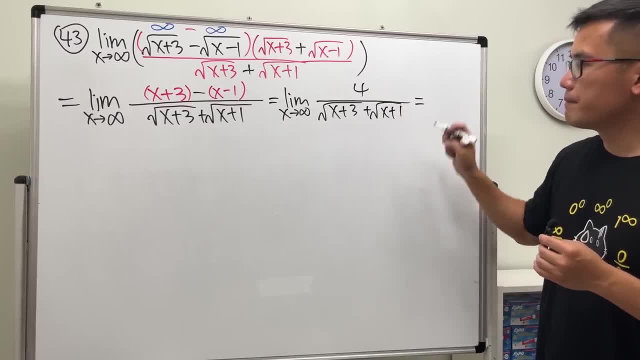 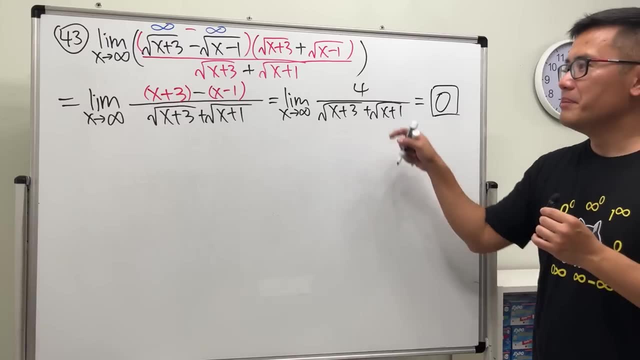 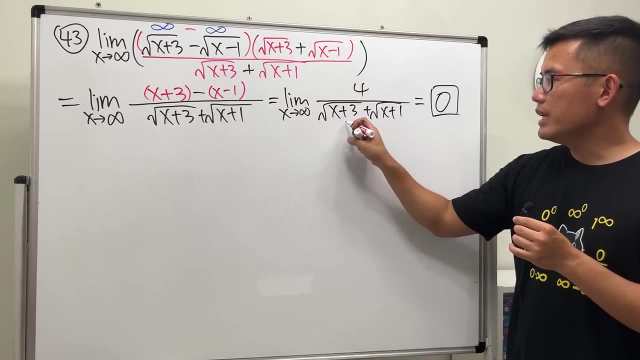 plus square root of x plus 1.. What's the answer for this? 0. Why? Because the top, as you can see, is just a 4, it's finite. But if you have the infinity on the bottom, you will get infinity plus infinity which. 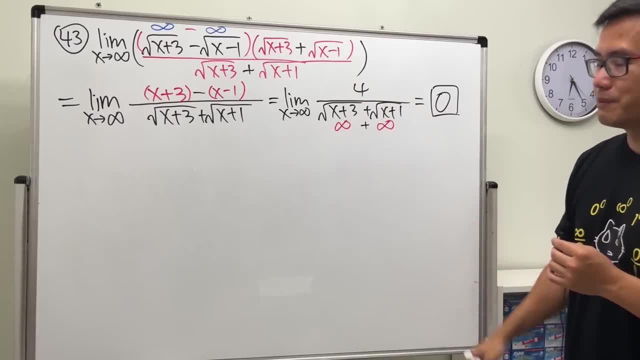 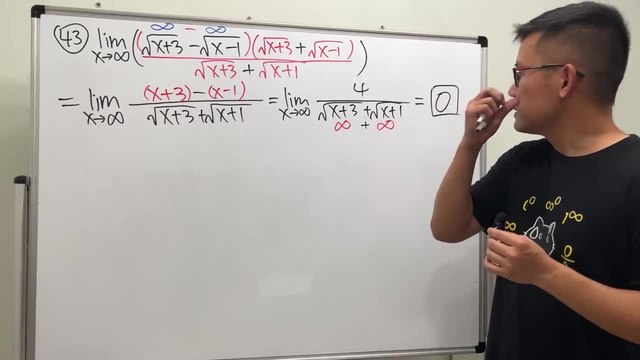 is infinity, 4 over infinity, we get 0.. Okay, so x minus x is gone. so yeah, cool huh. So in this case, yeah, my goodness, infinity minus infinity, we did get 0.. Did I say anything wrong? 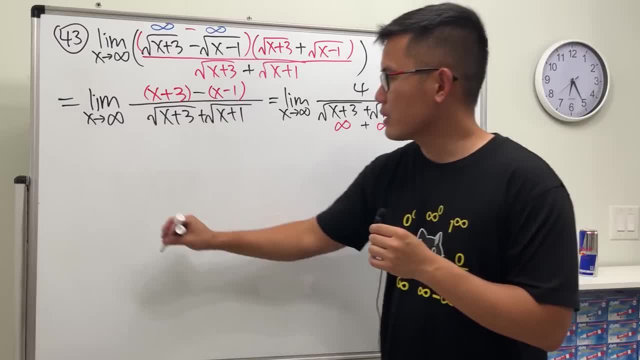 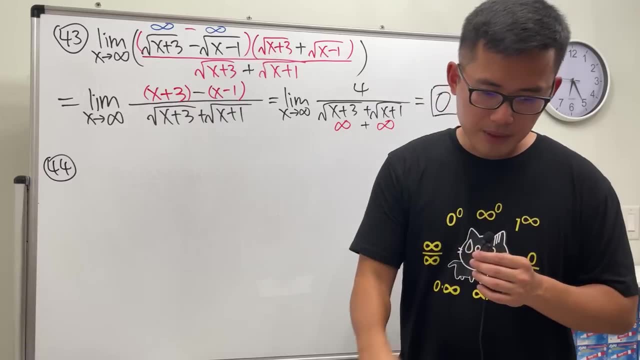 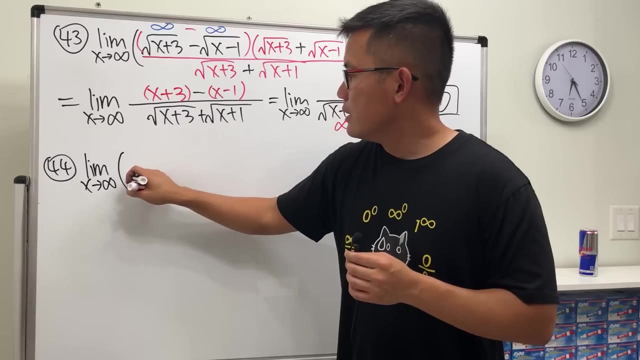 No, Don't worry, have a look. Let's look at number 44.. Oh, I'm going to change a little bit. huh, I'm just going to change a little bit. Let's look at the limit as x approaching infinity, square root of 2x plus 3, and then 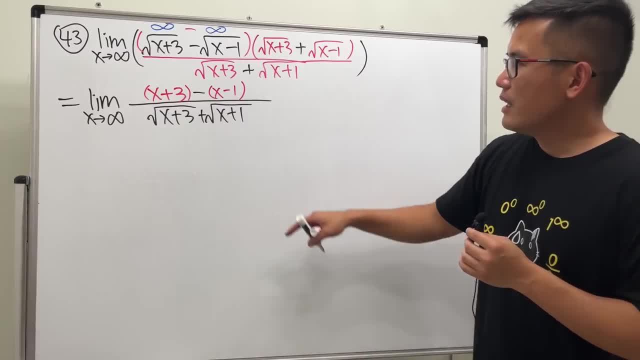 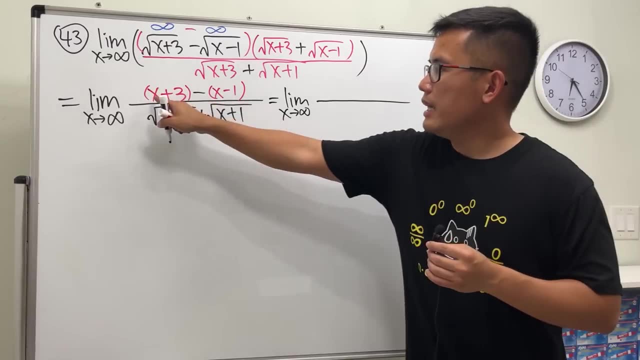 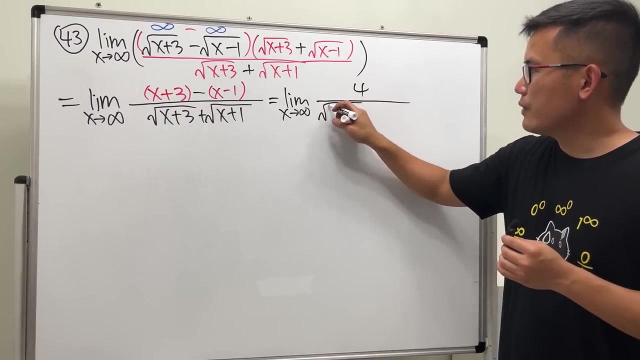 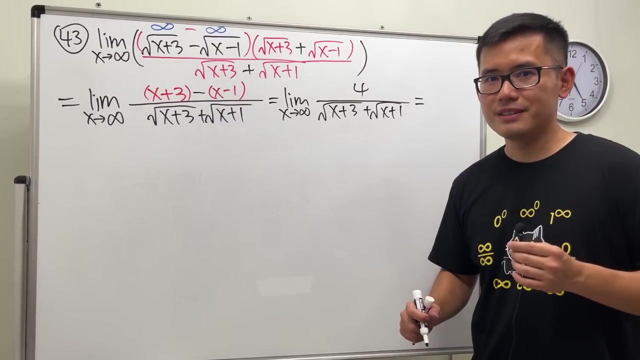 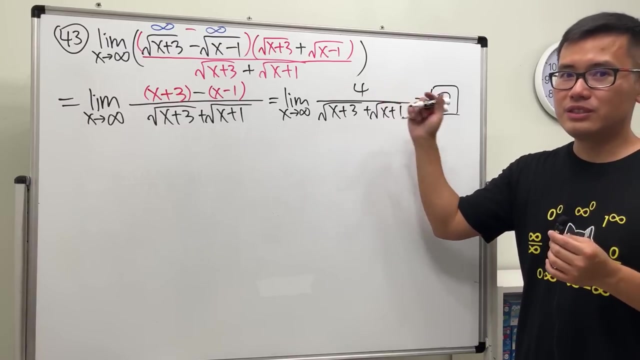 square root of X plus 3 plus square root of X plus 1, it doesn't matter. but second, pieимер and the SEC haveilanet tough. plus three plus square root of x plus one. what's the answer for this zero? why? because the top, as you can see, is just a four. it's finite. but if you have the infinity, 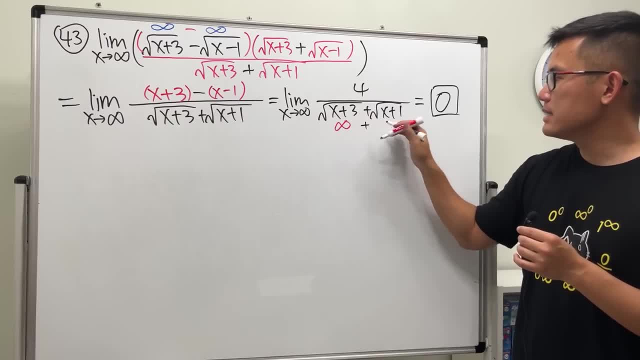 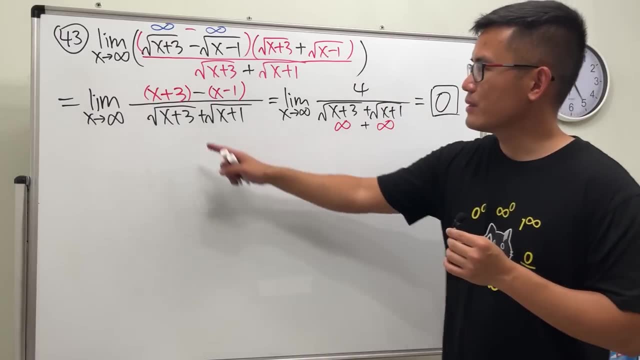 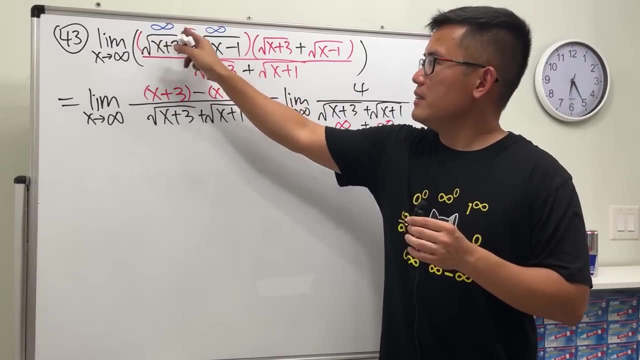 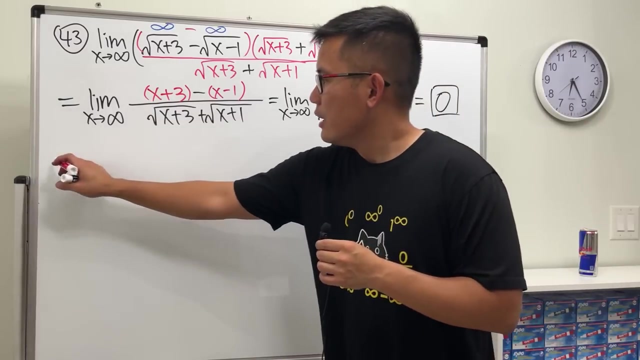 on the bottom, you will get infinity plus infinity, which is infinity four over infinity. we get zero. okay, so x minus x is gone. so, yeah, cool huh. so in this case, yeah, my goodness, infinity minus infinity, we take a zero. do you have anything wrong? don't worry, have a look. let's look at number 44. 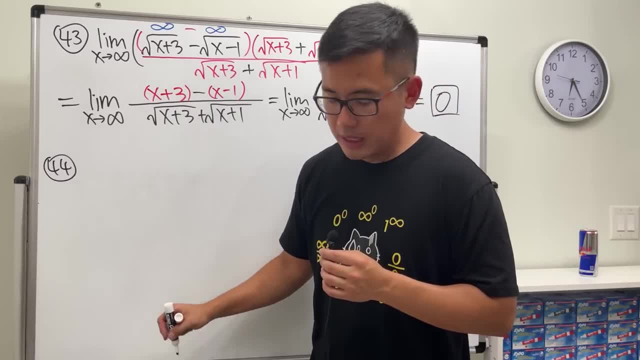 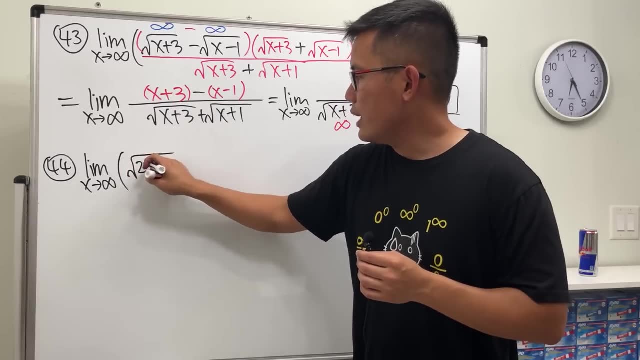 oh, i'm going to change a little bit. huh, i'm just going to change a little bit. let's look at the limit as x approaching infinity, squared root of 2x plus 3, and then minus square root of x minus 1, right? so I'm just 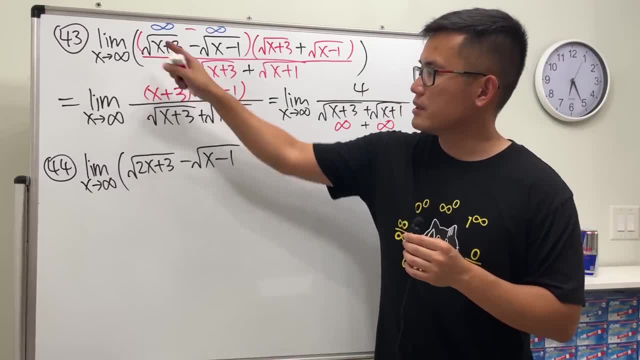 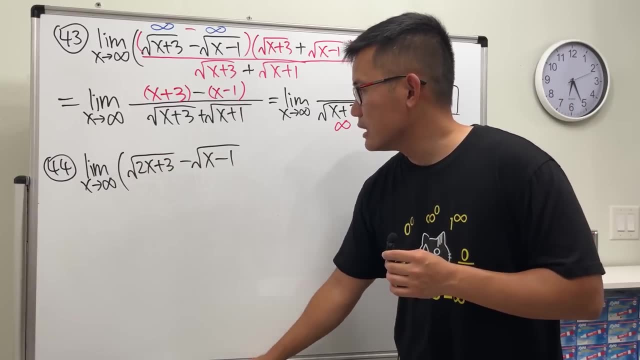 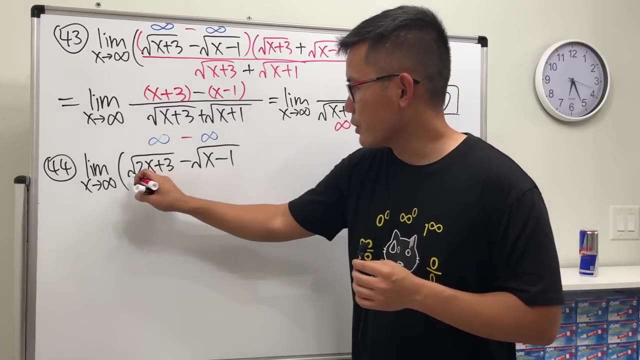 gonna change this a little bit. well, I have a 2 right here instead. okay, and the same idea. we also have infinity minus infinity, so I'm not going to say too much about it. we'll just go ahead and get to work. so, multiply the top and 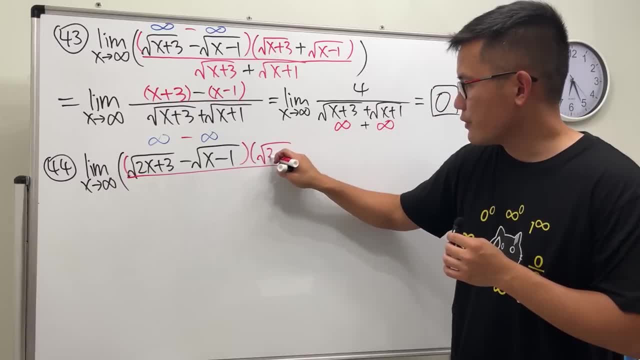 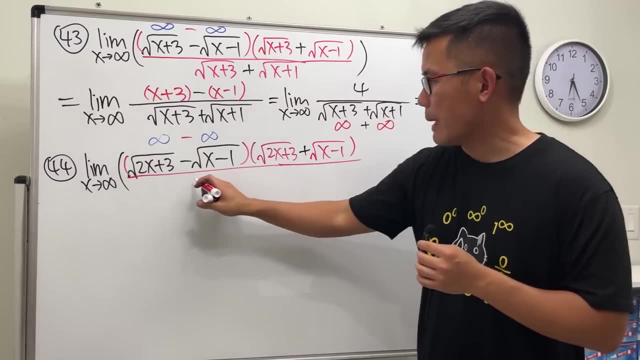 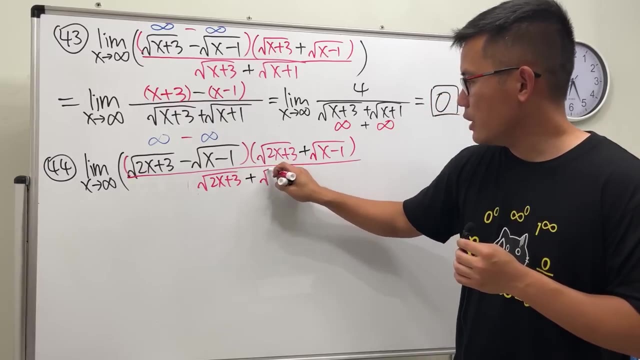 bottom by conjugate, which is square root of 2x plus 3 plus the square root of x minus 1, and then same thing on the bottom: square root of 2x plus 3, and then plus square root of x minus 1. cool, same thing on that, like earlier. here we have. 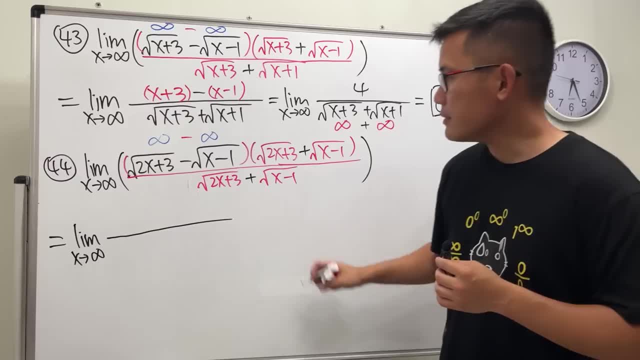 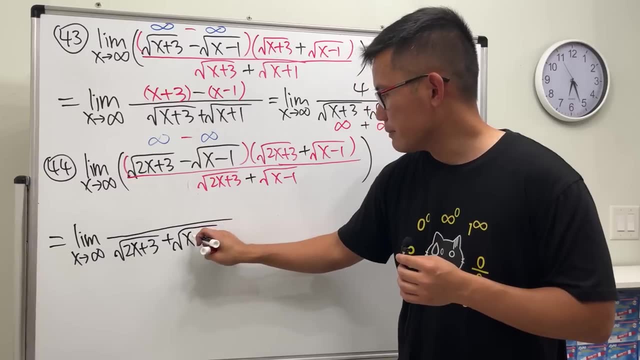 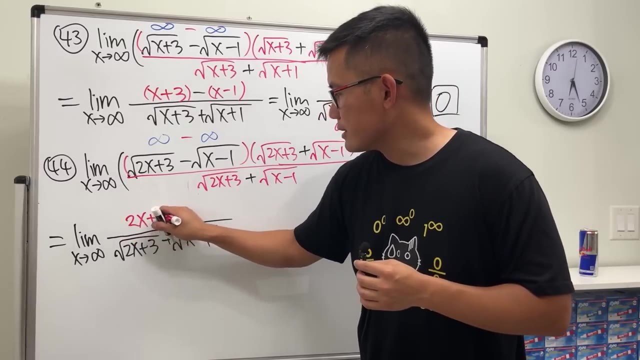 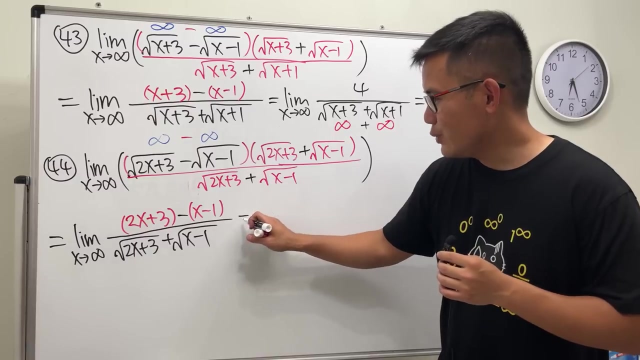 the limit as X approaching infinity. alright, so here we have square root of 2x plus 3 and then plus square root of x minus 1. what's on the top square? this minus square that? so we have 2x plus 3 and then minus x minus 1. okay, let's see. 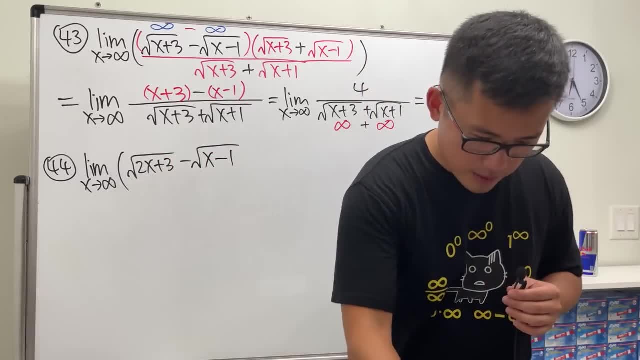 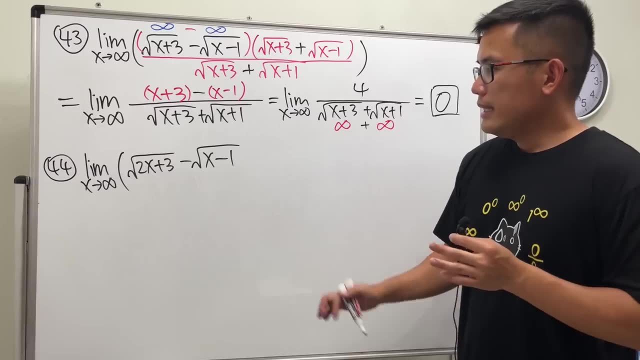 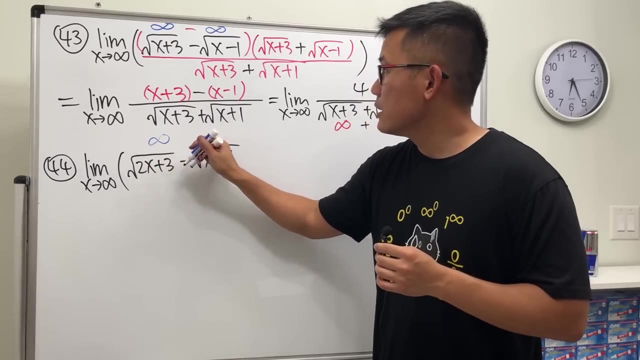 minus square root of x minus 1.. Alright, so I'm just going to change this a little bit. Well, I have a 2 right here instead, And it's the same idea. We also have infinity minus infinity, so I'm not going to say too much about it. 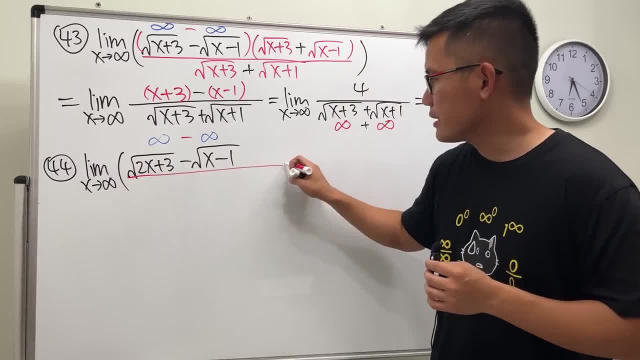 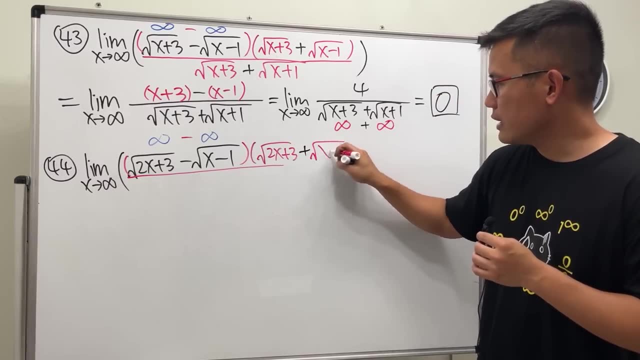 We'll just go ahead and get to work. So multiply the top and bottom by conjugate, which is square root of 2x plus 3 plus square root of x minus 1.. And then same thing on the bottom Square root of 2x plus 3.. 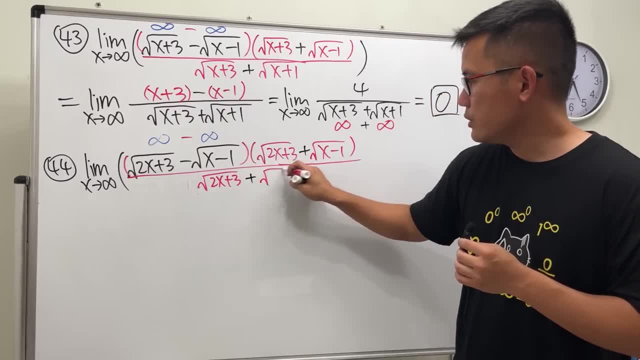 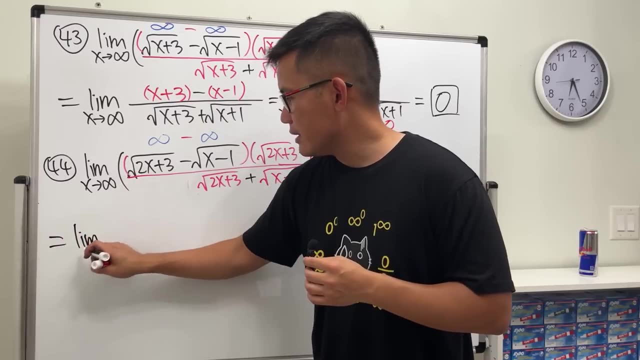 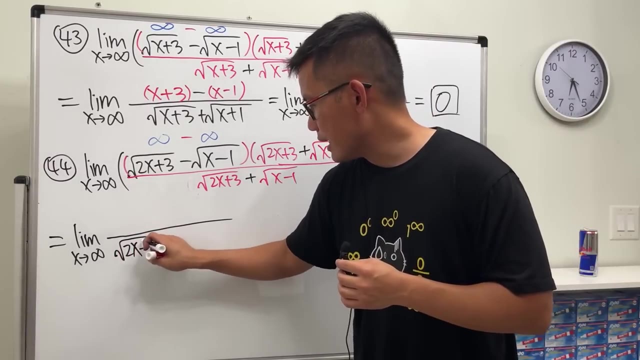 And then minus x minus 1.. Okay, And then plus square root of x minus 1.. Cool, Same thing like earlier. Here we have the limit as x approaching infinity. Alright, so here we have square root of 2x plus 3, and then plus square root of x minus. 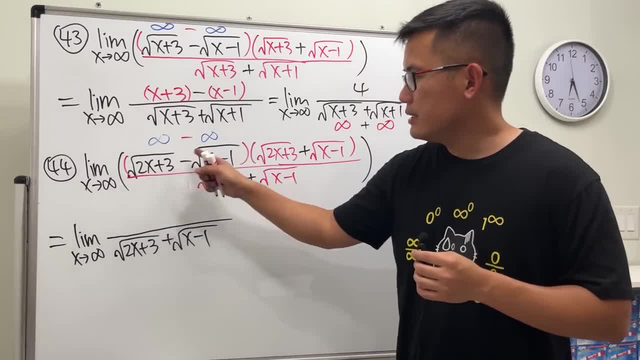 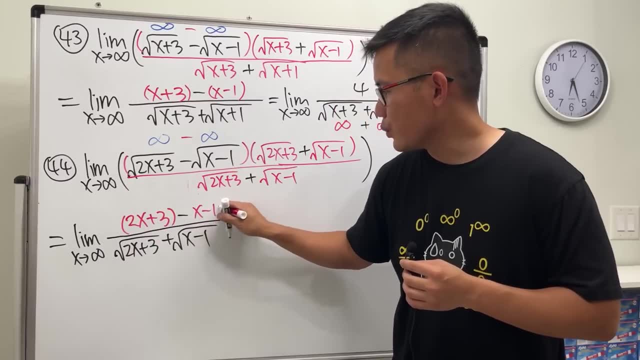 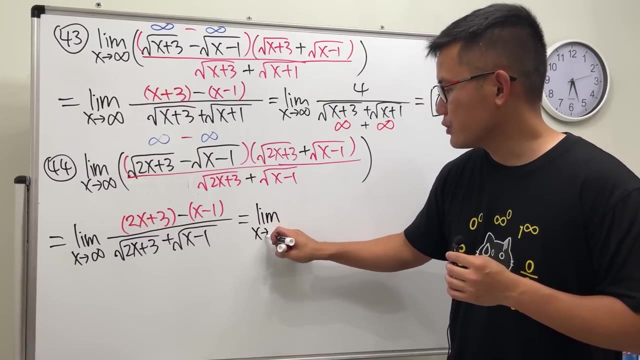 1. What's on the top Square? this minus square that. So we have 2x plus 3. And then minus x minus 1. Okay, Let's see what exactly we are going to get this time. This is the limit as x approaching infinity. 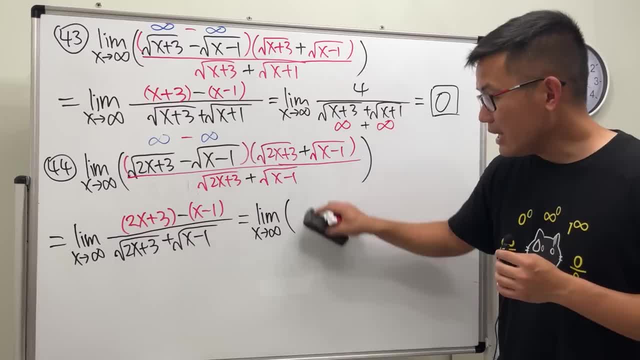 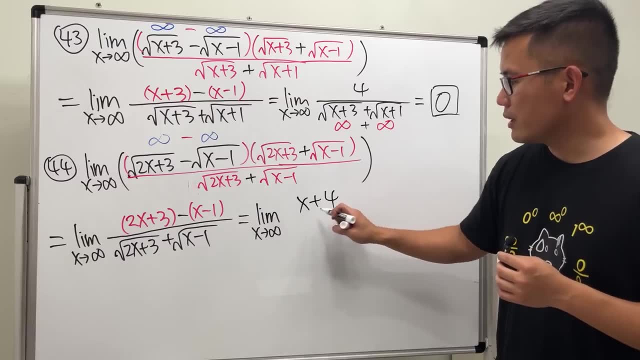 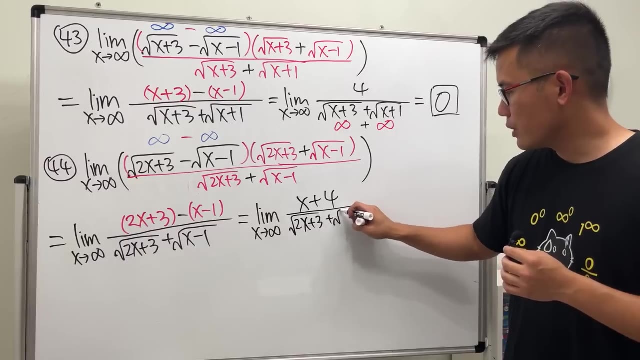 X. sorry, 2x minus x is x, So we have x on the top now. huh, Three minus negative 1 is 4, and that's a positive 4.. So it's x plus 4 over those things, Square root of 2x plus 3 plus square root of x minus 1.. 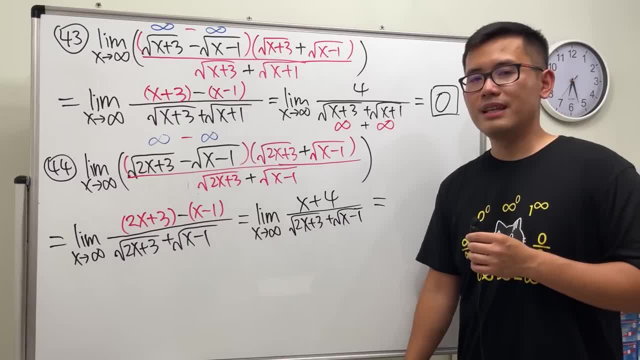 Okay, Okay. So what's the answer this time? What's the answer this time? I'll tell you The answer for this one, right here, is infinity. I'll tell you The answer for this one, right here, is infinity. I'll show you. 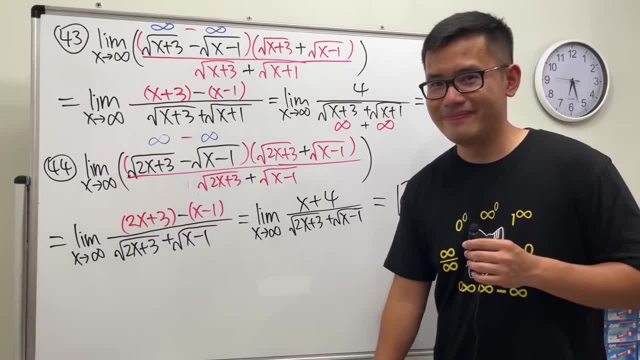 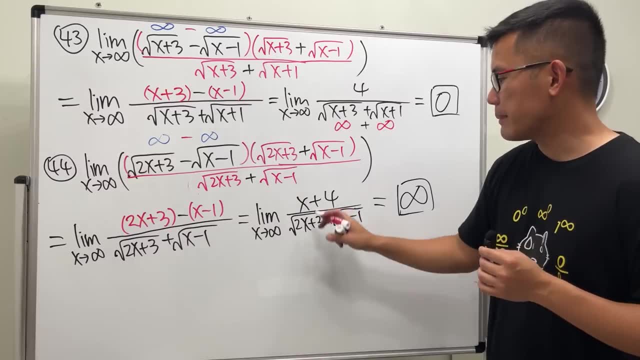 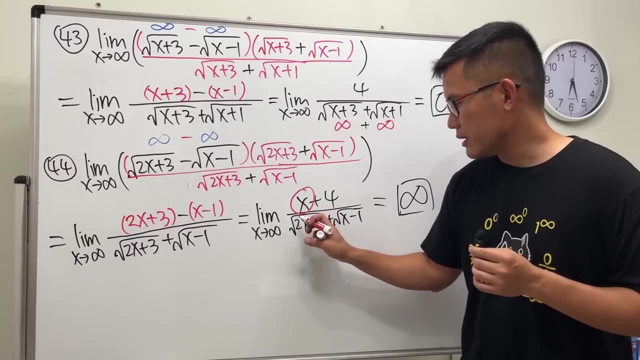 Alright, Again, x is approaching infinity. so picked up the dominating part on the top, which is just x to the first power On the bottom. picked up the dominating part, the plus 3, doesn't matter. so we have square root of 2x. 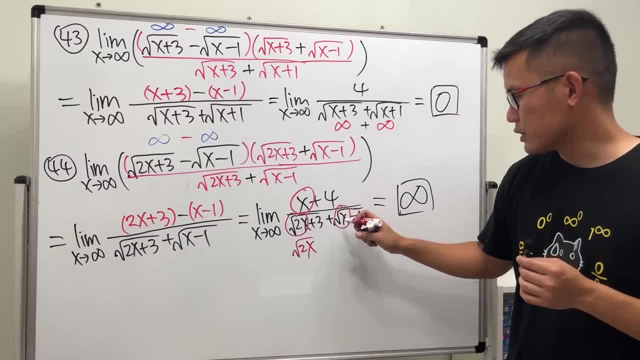 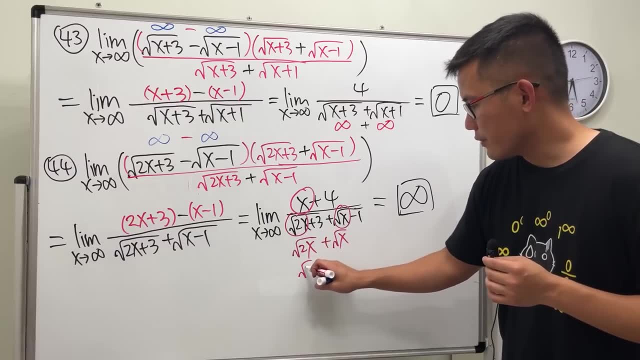 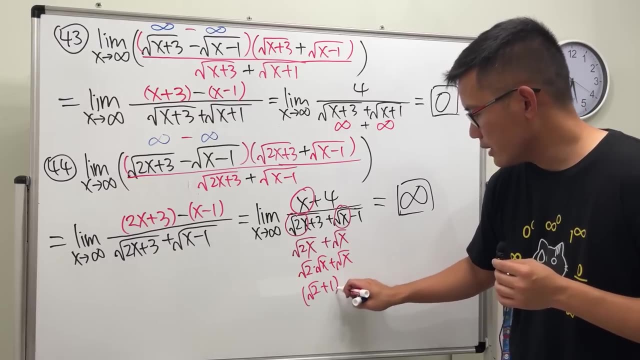 Okay, Okay, Okay. So we also have the square root of x. Yeah, So technically we can look at this as the square root of 2 times square root of x plus square root of x, and we can combine them as the square root of 2 plus 1 times square. 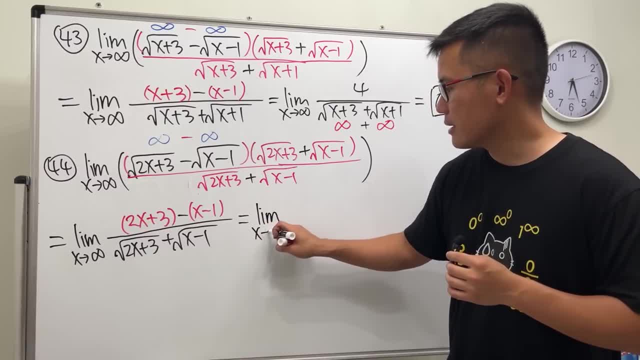 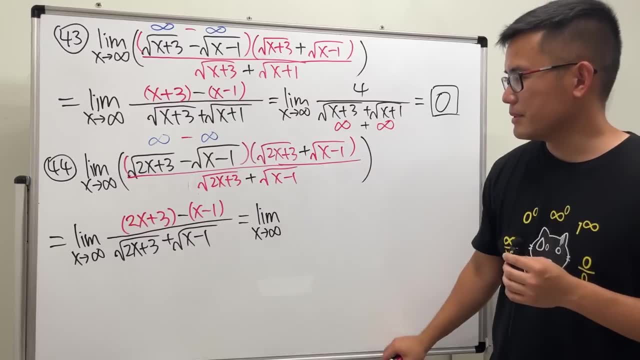 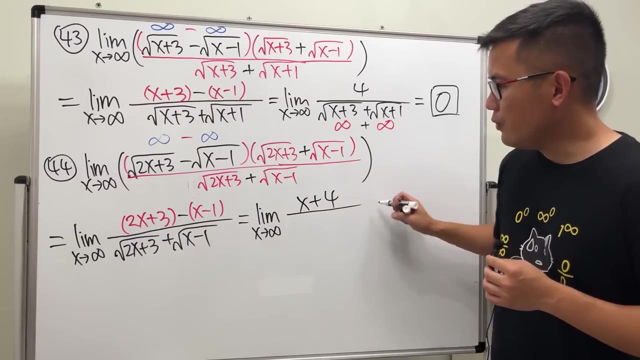 what exactly we are going to get this time. this is the limit as X approaching infinity X. sorry, 2x minus X is X, so we have X on the top now. huh, 3 minus negative 1 is 4 and that's a positive 4, so it's X plus 4. over those. 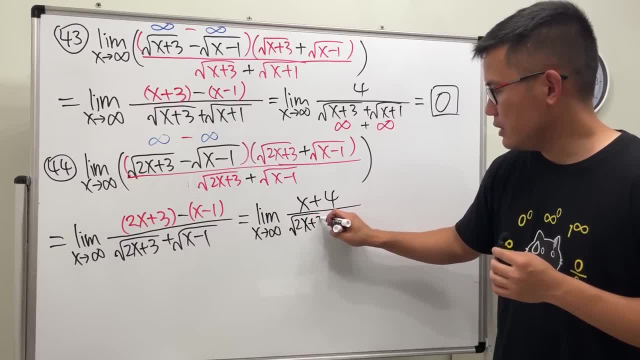 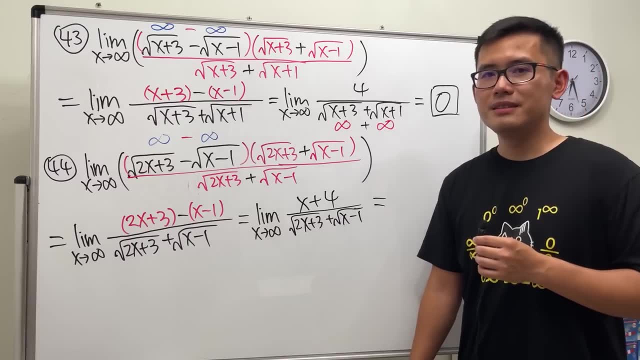 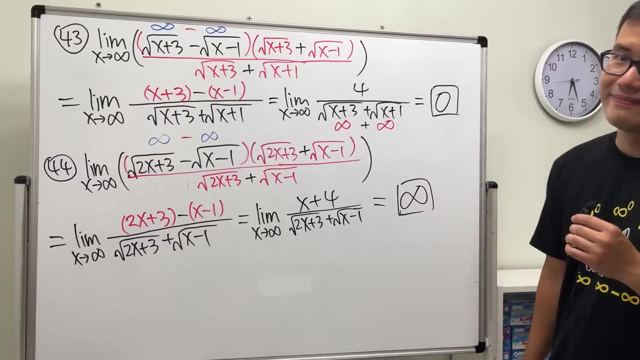 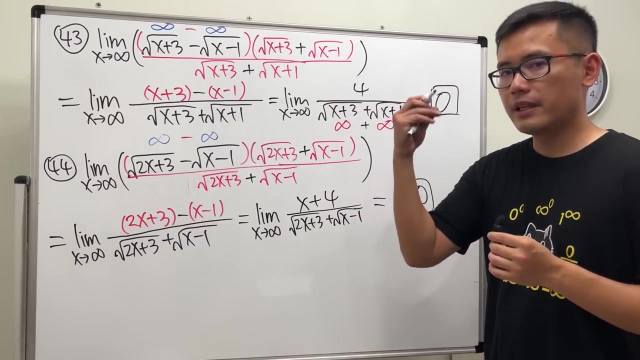 things: square root of 2x plus 3 plus square root of X minus 1. what's the answer this time? I'll tell you the answer for this one, right here, is infinity. all right, again, X is approaching infinity, so picked out the dominating part on the. 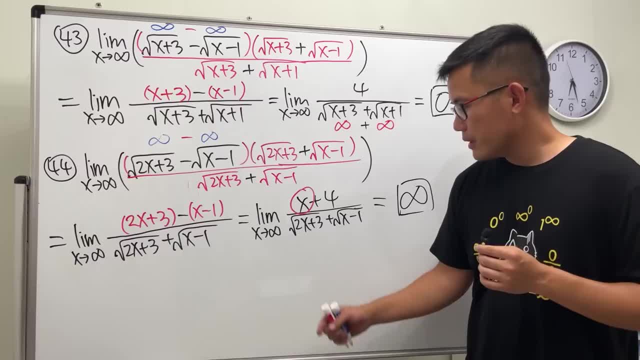 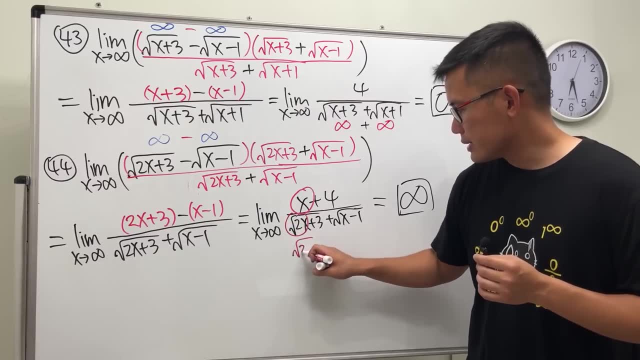 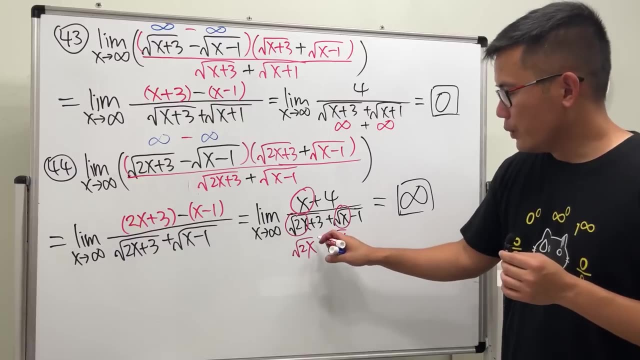 top, which is just X, to the first power at the bottom picked out the dominating part, the plus 3. doesn't matter if we have square root of 2x and then from this we also have the square root of X. ya, so technically we can look at this as: 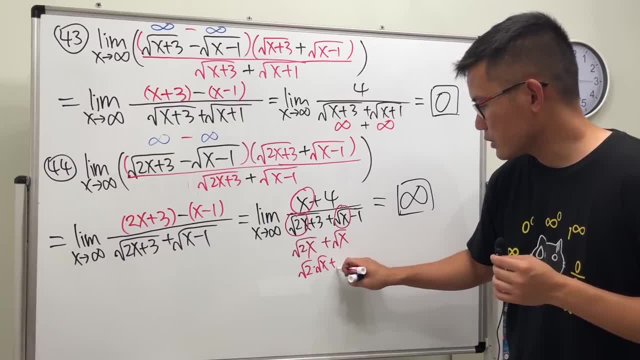 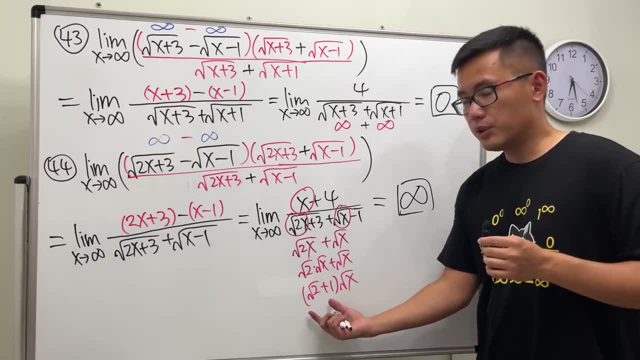 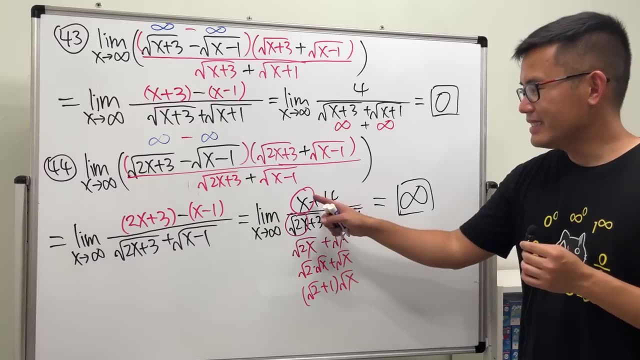 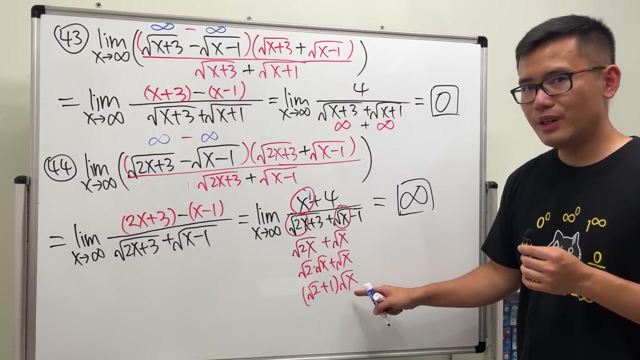 square root of 2 times square root of X plus square root of X, and we can combine them as squared with a 2 plus one times square root of x. this is just a coefficient, but the main thing is we have x over that. this is x to what power? this is x to the first power. this is x to the one half power. 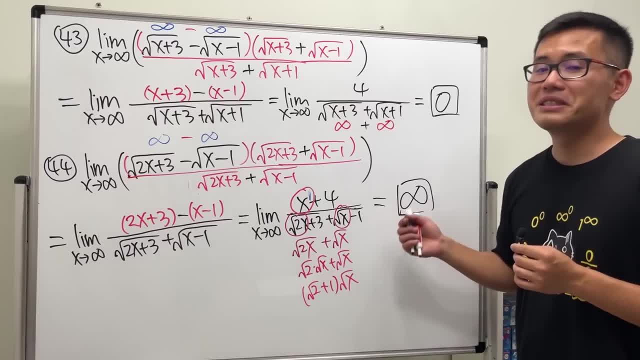 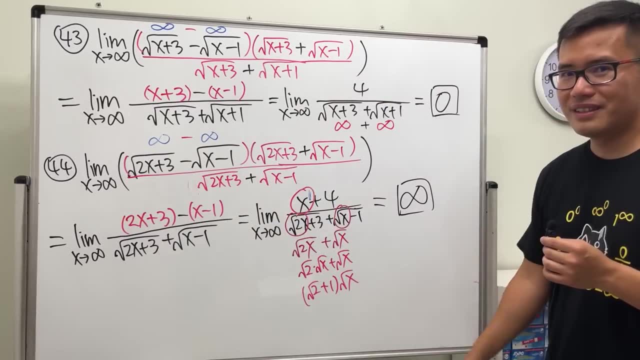 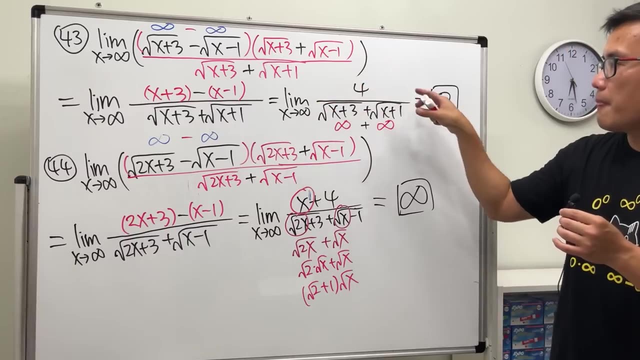 which one's bigger top is bigger whole thing is infinity, told you, and, as you can see, infinity minus infinity. hey, we end up with infinity. all right, quick summary: the number 33, we get 0. the answer for number 33 is 0. this tells us this expression and that 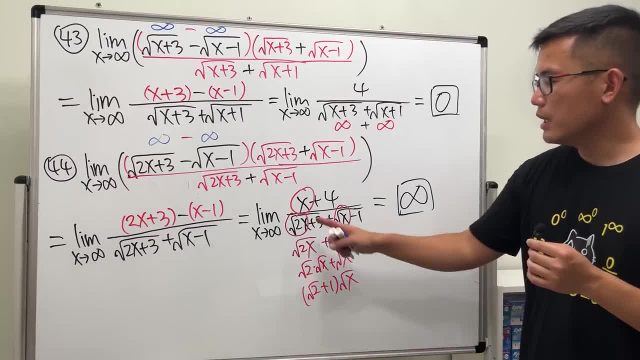 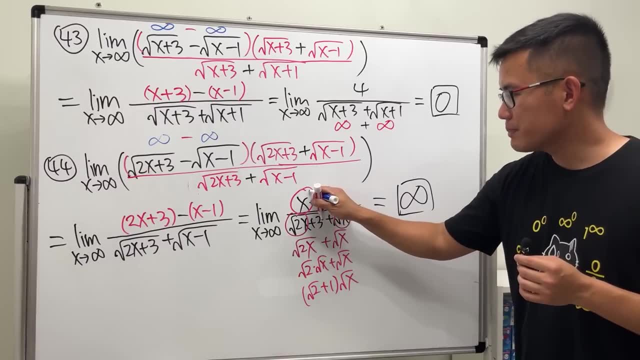 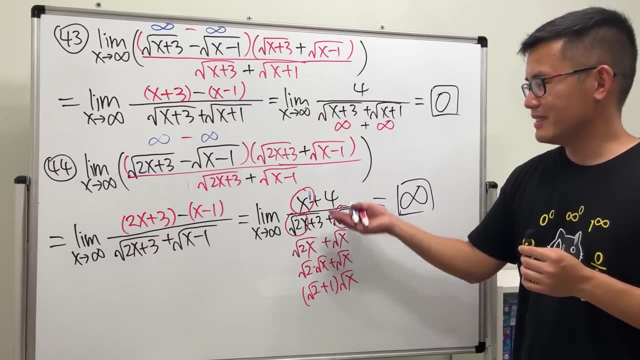 root of x. This is just a coefficient, but the main thing is we have x over that. This is x to 1 power. This is x to the first power, This isaeda, this is x to the 1 half power. which one's bigger top is bigger whole thing. 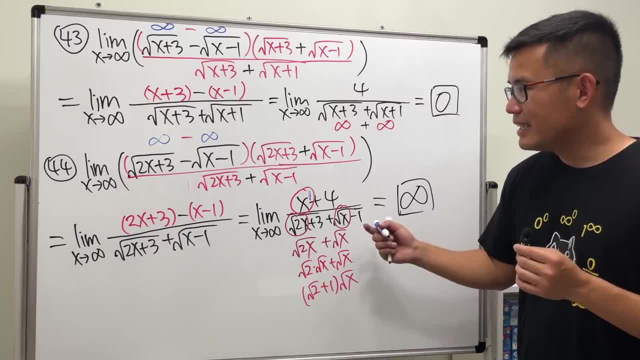 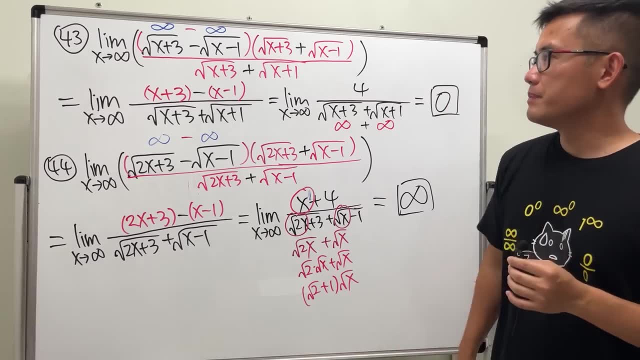 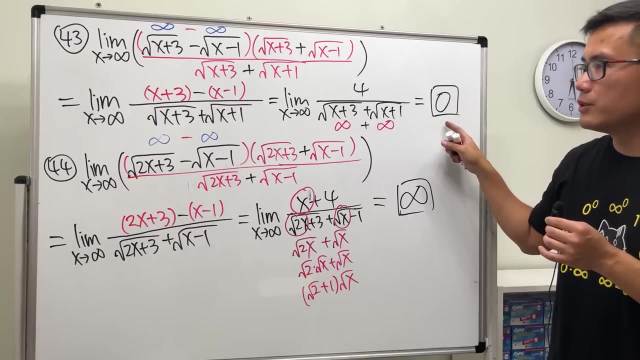 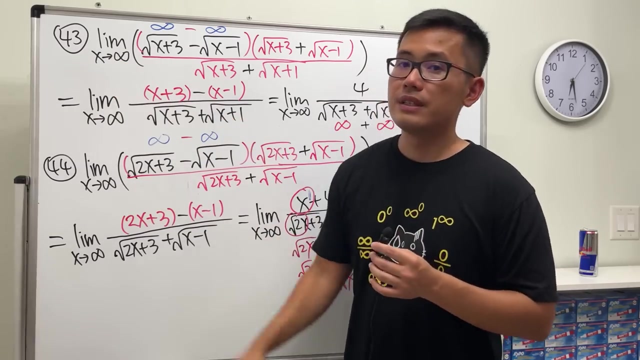 is infinity, told you, and, as you can see, infinity minus infinity a, we end up infinity. all right, quick summary: the number 33 we guess you wrote the answer for number 33 is 0. this tells us this expression and expression are about the same size as X goes to infinity. okay, however, the answer for number 44 is: 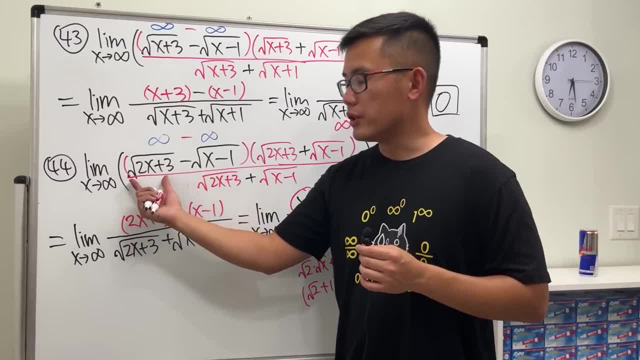 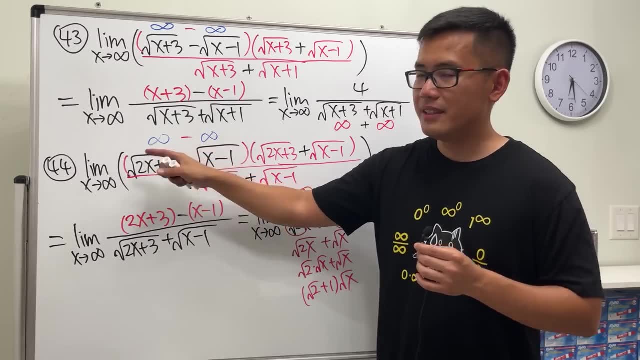 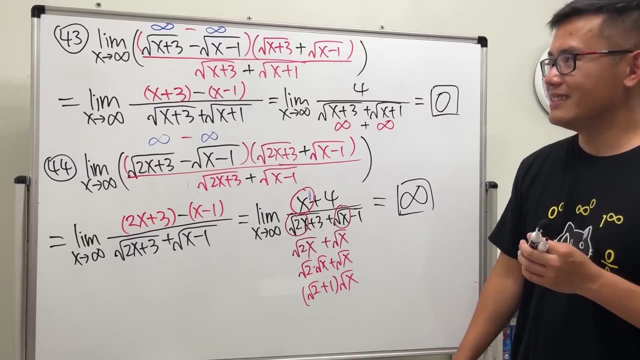 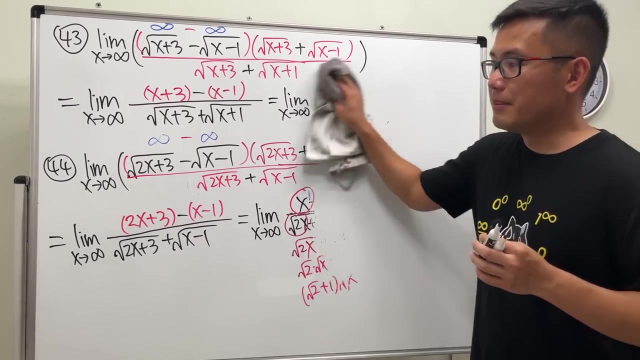 equal to infinity. it means this expression is so, so, so much bigger than that, as X goes to infinity. so that's why, when you subtract this, infinity is way bigger than that. so not only the vanities are the same size. yeah, all right, I'm also going to show you guys number 45. it's another infinity minus infinity. 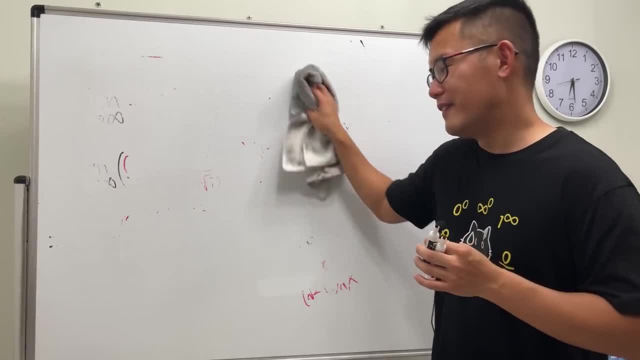 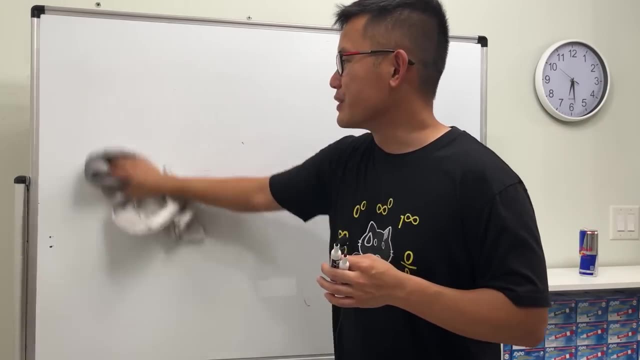 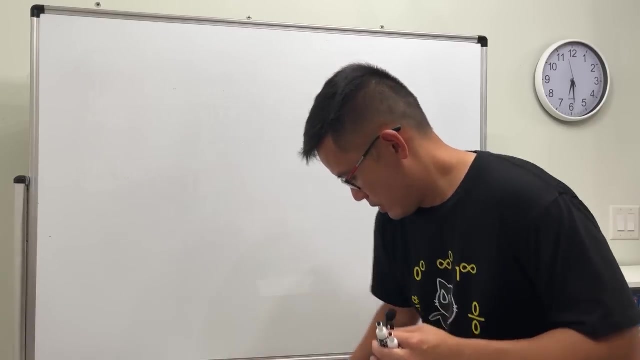 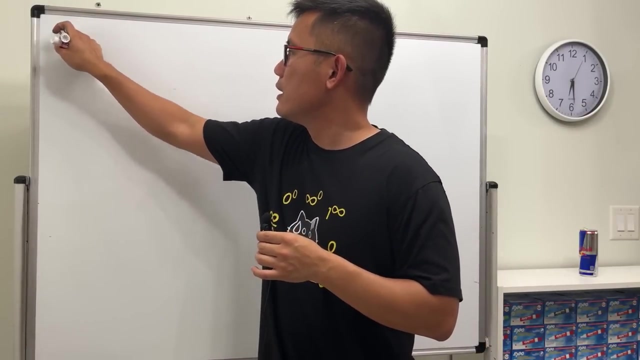 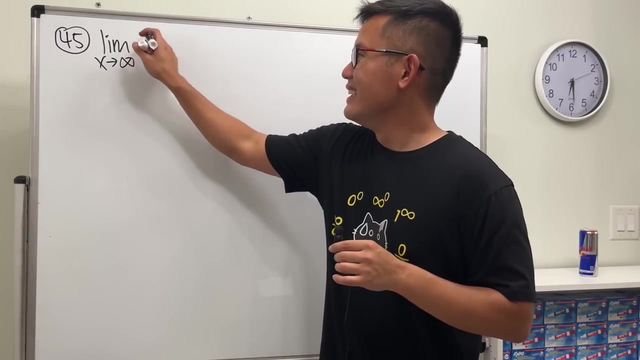 situation and we will actually get a very interesting value. it's a finite value. it's not like a super cool number like e to the square root of 17 for something. no, it's just, you'll see, number 45. here we have the limit S, X approaching infinity, and then square root of x. 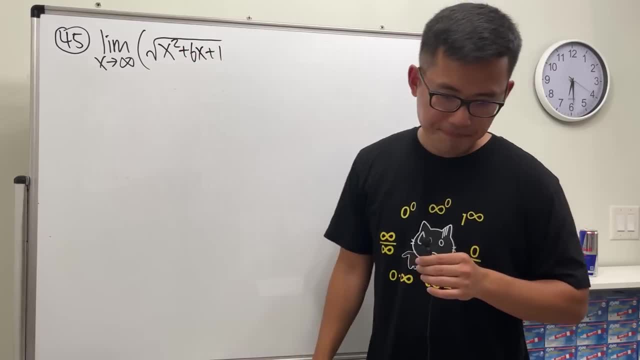 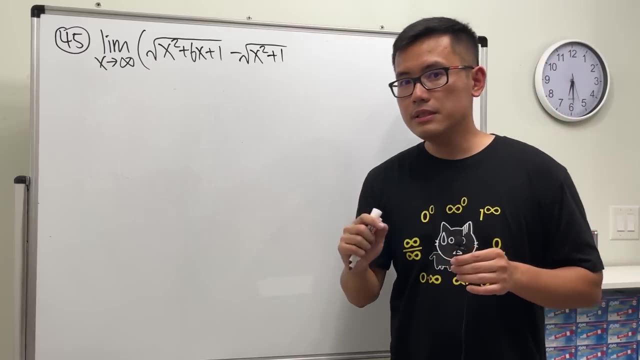 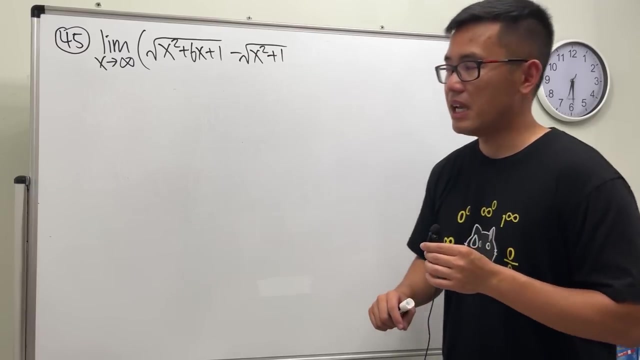 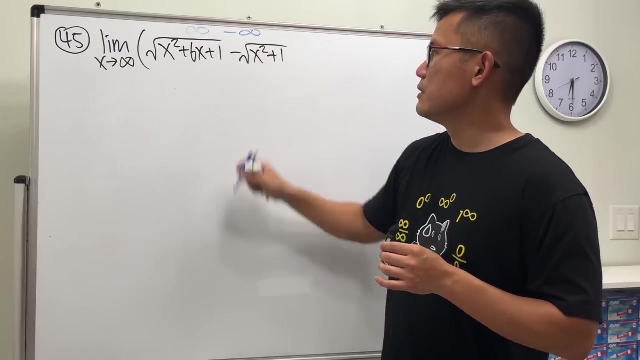 squared plus 6x plus 1, and the minus square root of x squared plus 1, and notice this time the inside. here they are both quadratic earlier, they are just both linear. yeah, anyway, if you put infinity into this and that we get infinity minus infinity, all right. so just want to mention that real quick. but 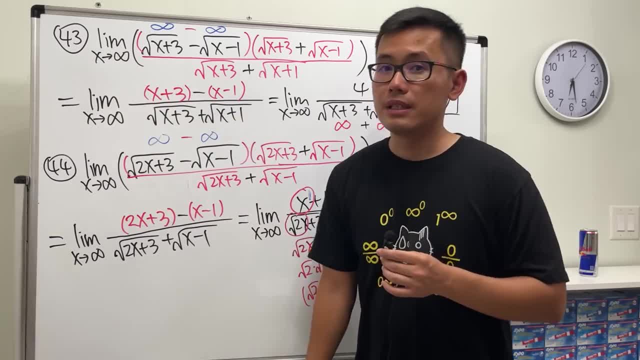 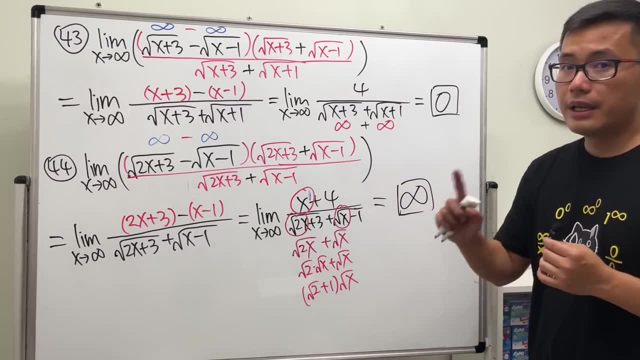 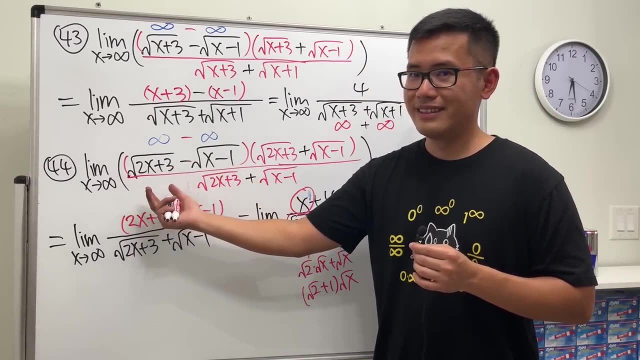 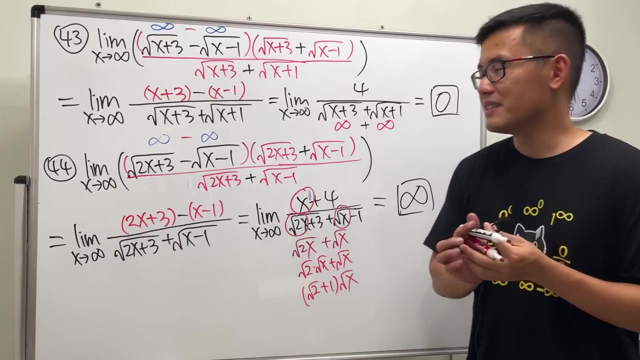 expression are about the same size as x goes to infinity. okay. however, the answer for number 44 is equal to infinity. it means this expression is so, so, so much bigger than that as x goes to infinity. so that's why, when you subtract this, infinity is way bigger than that. so not all infinities are the same size. yeah, 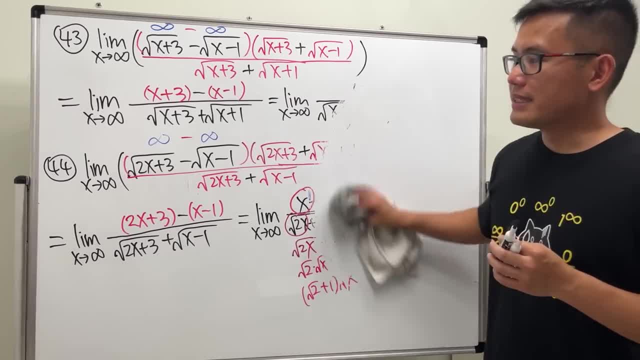 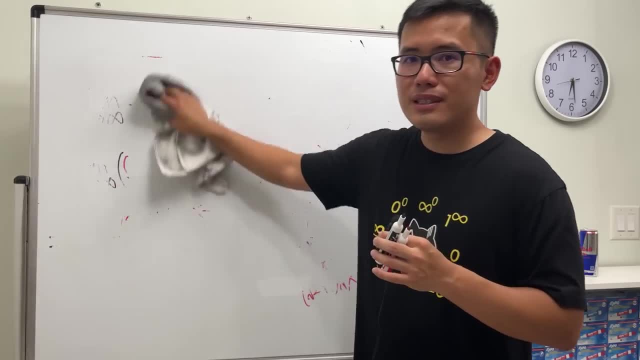 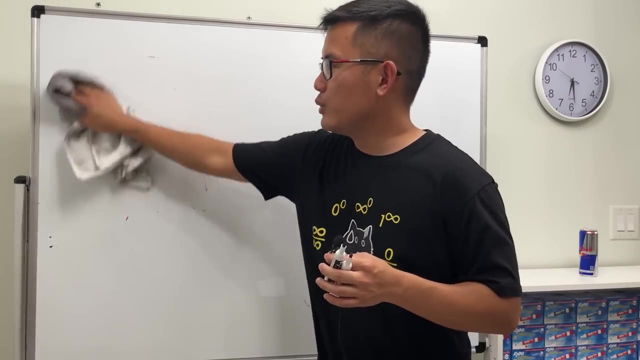 all right, i'm also going to show you guys number 45. it's another infinity minus infinity situation and we will actually get a very interesting value. it's a finite value. it's not like a super cool number, like e to the square root of 17 for something, no, it's just. you'll see, 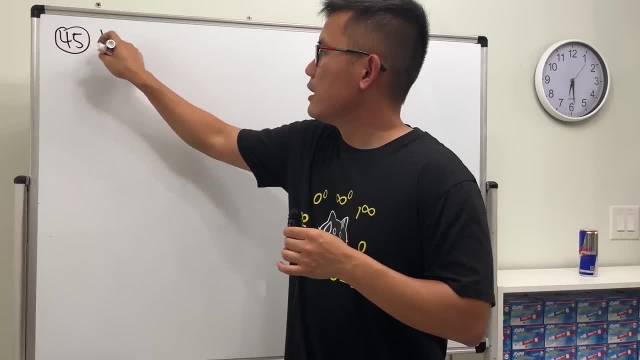 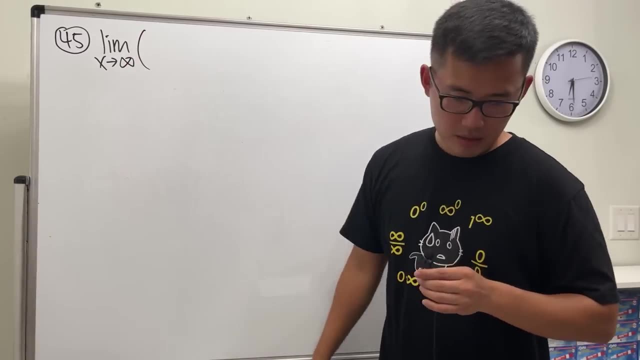 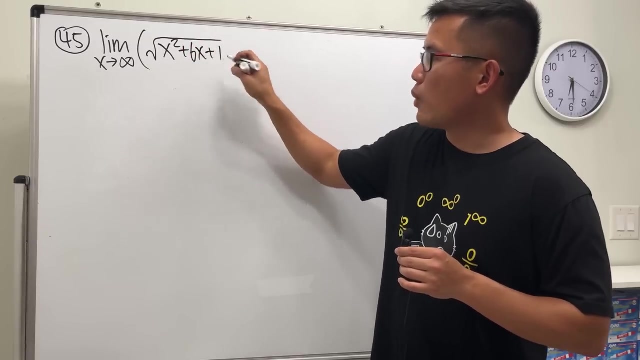 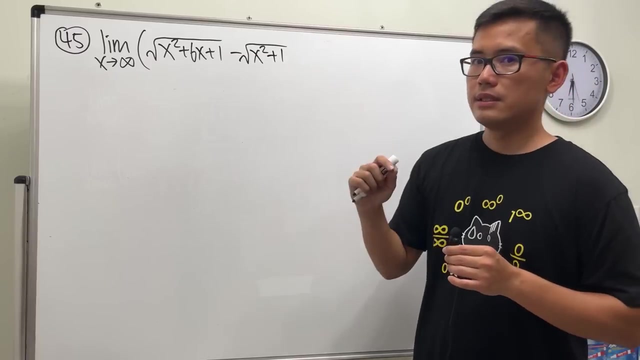 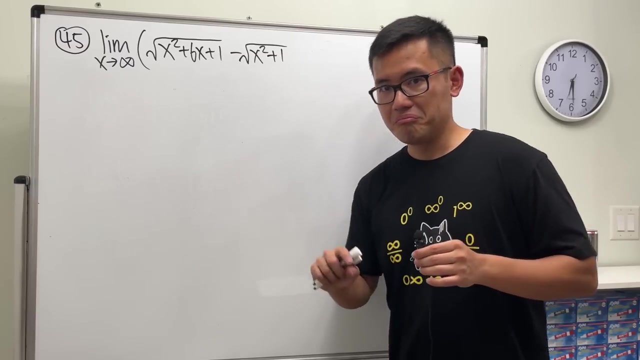 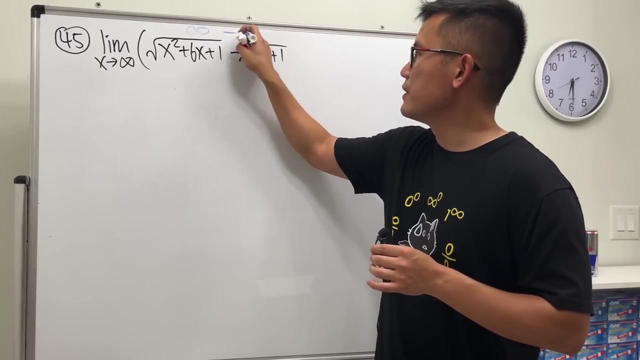 number 45. here we have the limit as x approaching infinity, and then square root of e to the square root of 17, and then minus sin, sin. so this will add up to x square plus 6x plus 1, and then minus square root of x square plus 1.. and notice this time: 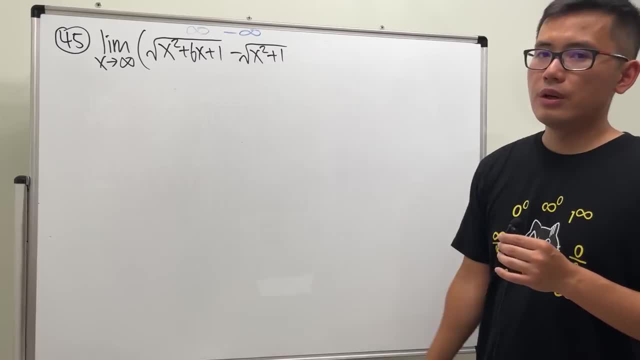 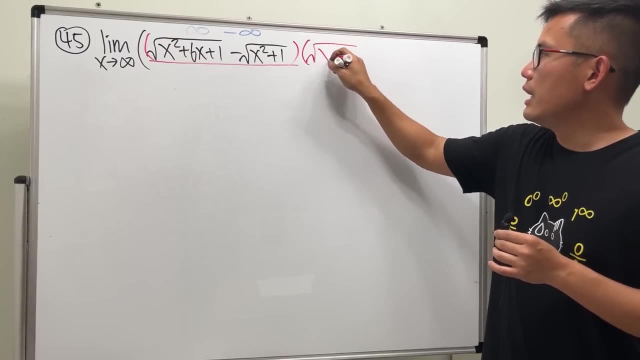 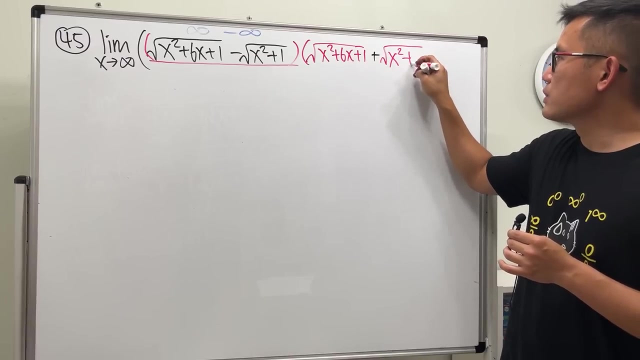 the inside. here they are both quadratic. earlier they are just both linear. yeah, anyway, if you put that, we will just multiply by the conjugate. So let's go ahead and just get to work. So square root x squared plus six, x plus one, and then plus square root of x squared plus one. 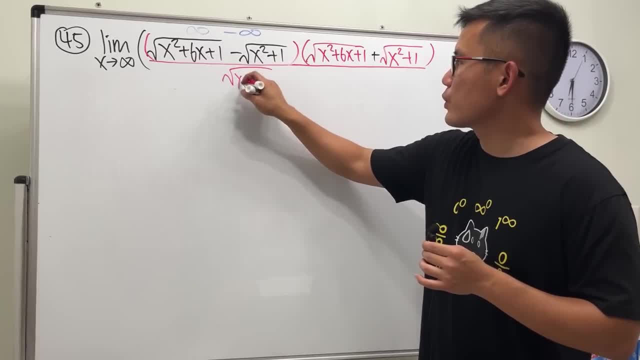 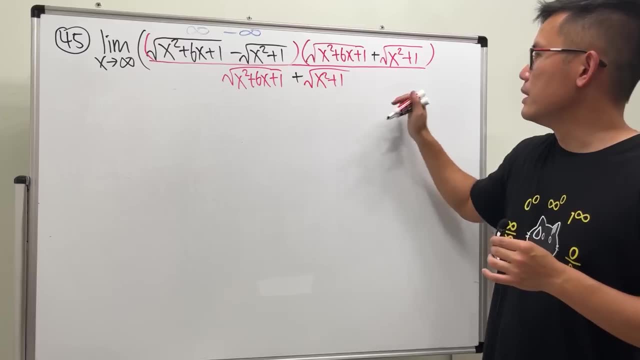 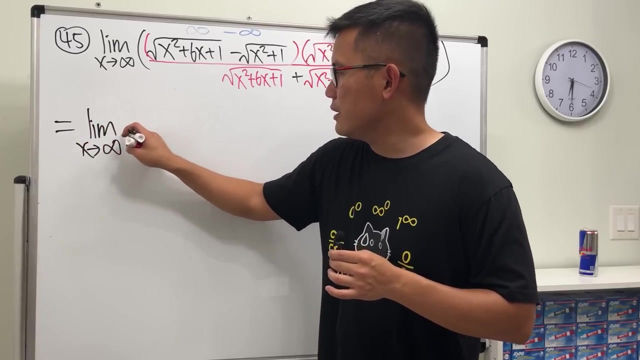 over the same thing. So square root of x squared plus six, x plus one, and then plus square root of x squared plus one. Okay, this right here gives us the limit as x approaching infinity. On the bottom, we have square root of x squared. 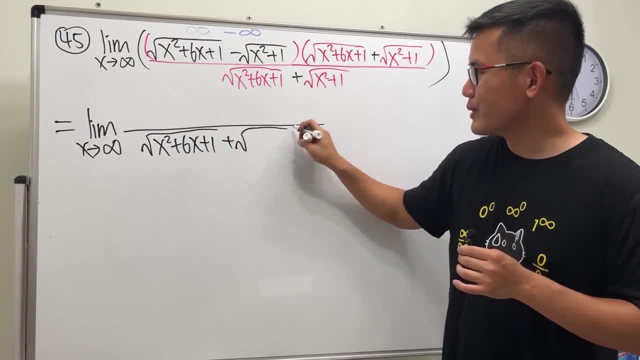 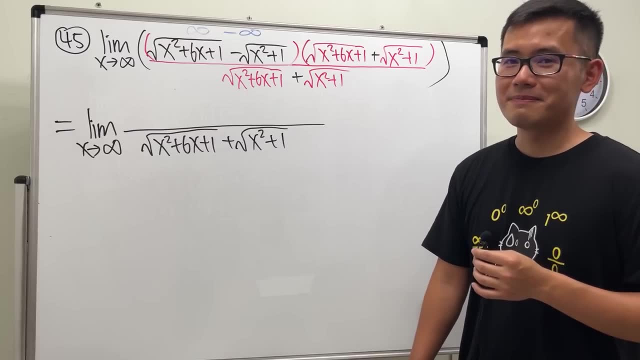 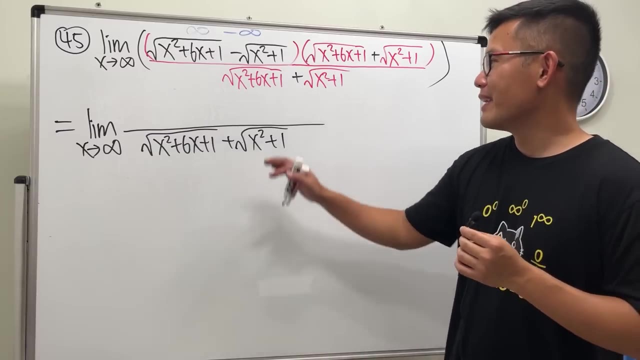 plus six, x plus one plus another square root of x squared plus one. You know why calculus is hard? It's because a lot of times we just have to write the same thing over and over and over. yeah, But anyway, though, bring this down now, multiply this out. 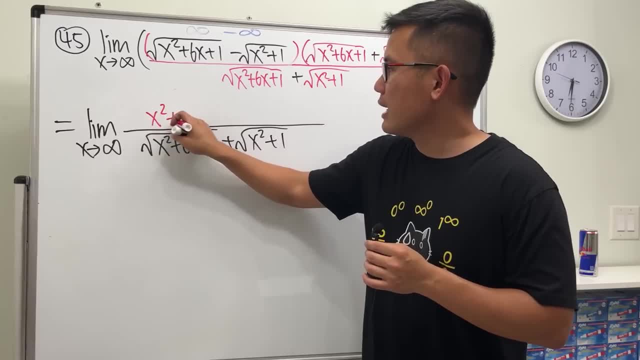 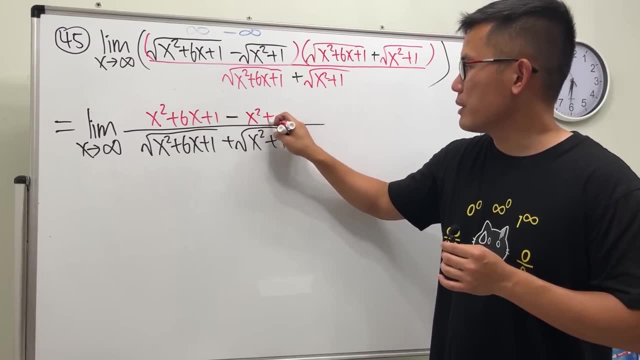 which shows how to square this, which is just x squared plus six, x plus one- You don't need parentheses for that- but then minus. you do need parentheses for this. x squared plus one. all right, So now check this out. 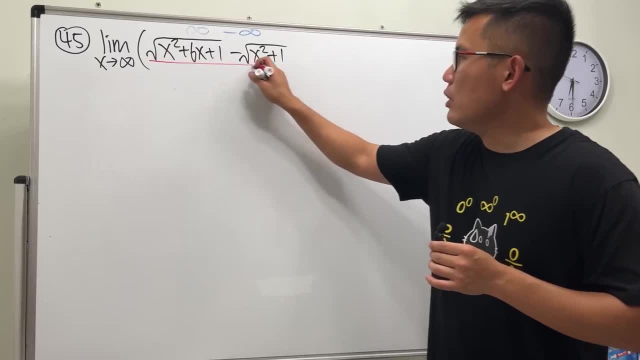 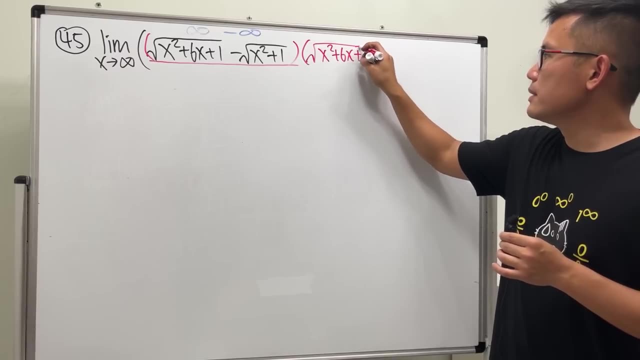 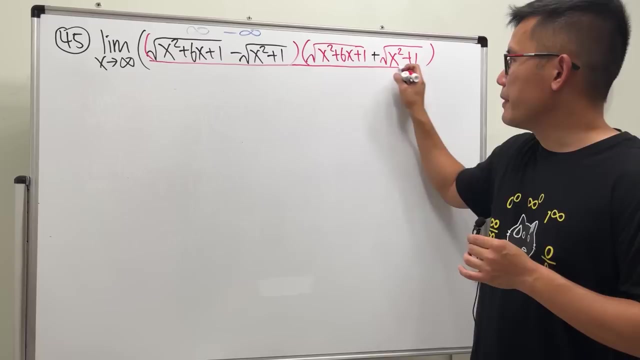 you know, the deal is that we will just multiply by the conjugate. so let's go ahead and just get to work. so square root x squared plus 6x plus 1, and then plus square root of x squared plus 1 over the same thing, so square root of x. 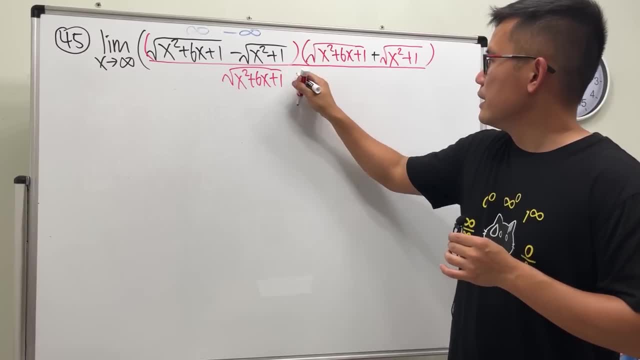 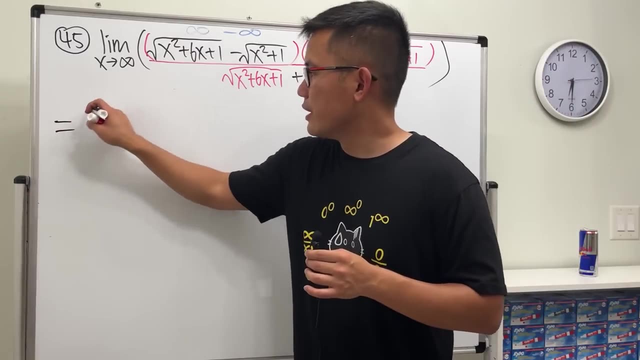 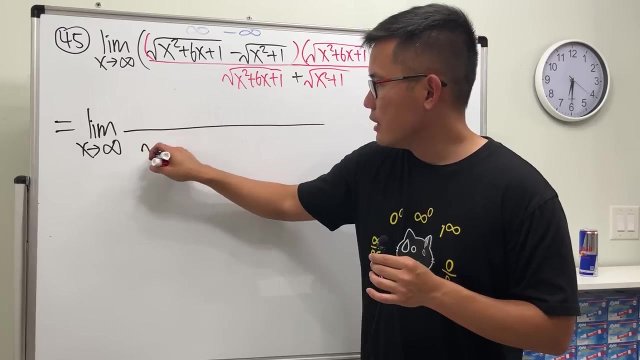 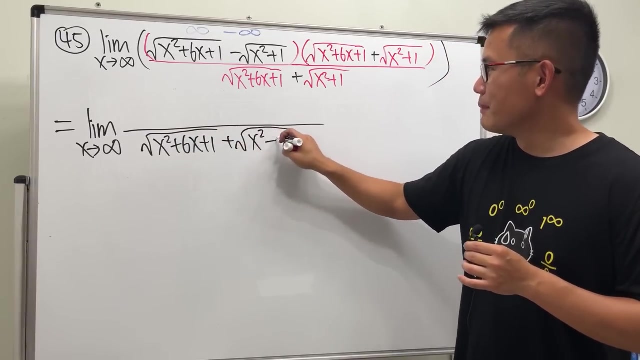 squared plus 6x plus 1, and then plus square root of x squared plus 1. okay, this right here gives us the limit as x approaching infinity. on the bottom we have square root of x squared plus 6x plus 1, plus another square root of x squared plus 1.. 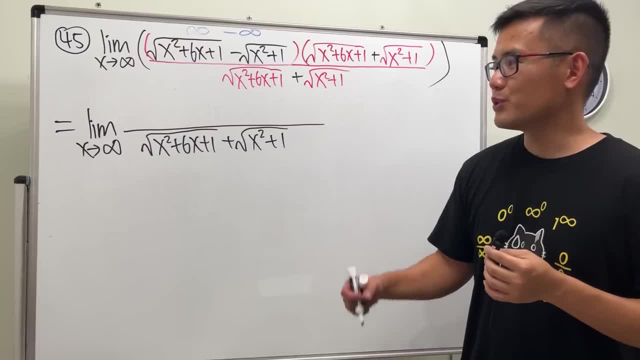 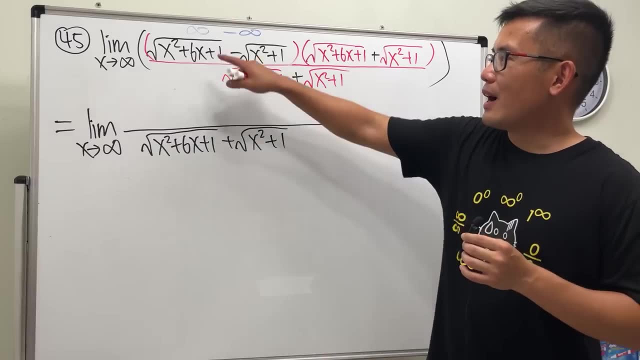 You know why calculus is hard? It's because a lot of times we just have to write the same thing over and over and over. Yeah, But anyway, though, bring this down Now, multiply this out. We just have to square this. 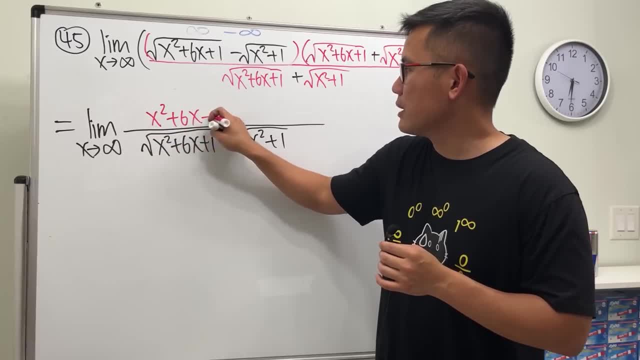 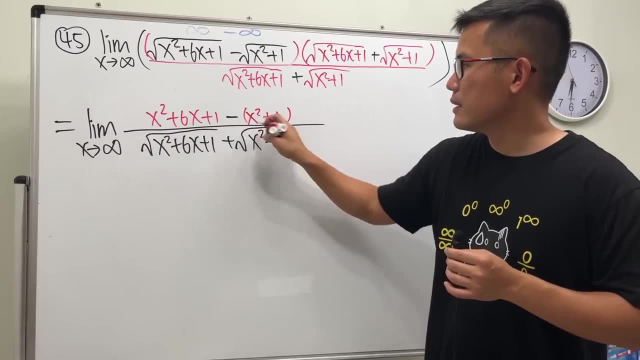 which is just x squared plus 6x plus 1.. You don't need a parenthesis for that, but in minus you do need a parenthesis, for this is x squared plus 1.. All right, So now check this out: x squared, x squared- they cancel. 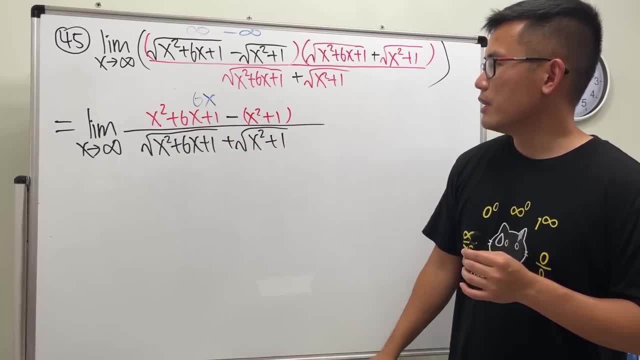 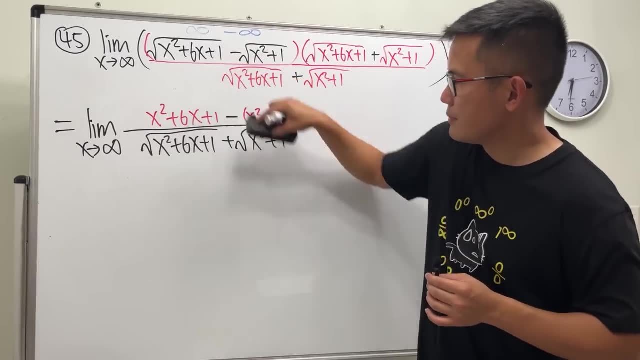 We have 6x on the top. Let me just put down the result here And then 1 minus 1.. I think I'm just going to rewrite everything again to make it super clear. So if we cancel the top, this is the limit as x approaching infinity. 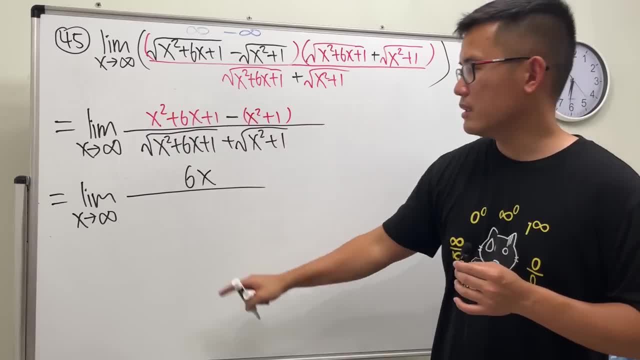 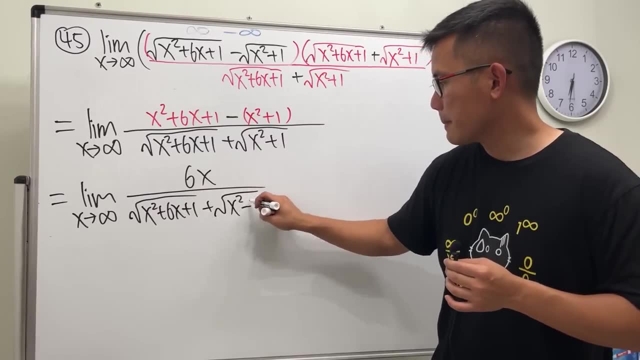 We will just get 6x on the top. 1 minus 1 is also gone, And then we just have to cancel all this. Okay, Picked up the highest power of x on the top. It's just this: 6x to the first power. 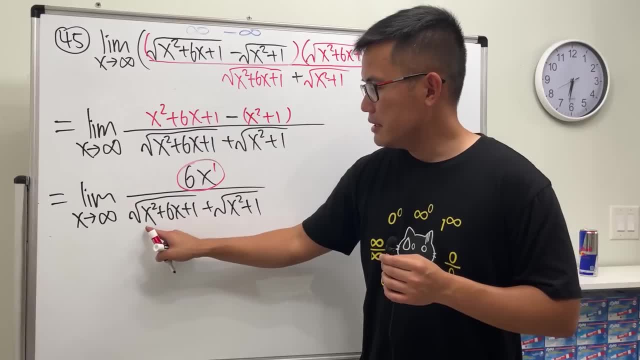 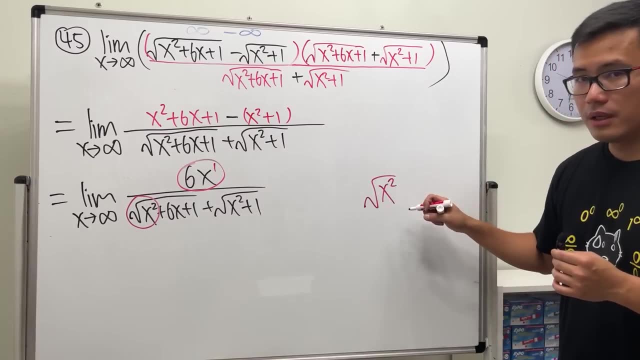 But guess what? On the bottom, this is the highest power, right here And square root of x squared. What's square root of x squared? Yes, we can cancel them, But if you just cancel them, you actually have to put an absolute value. 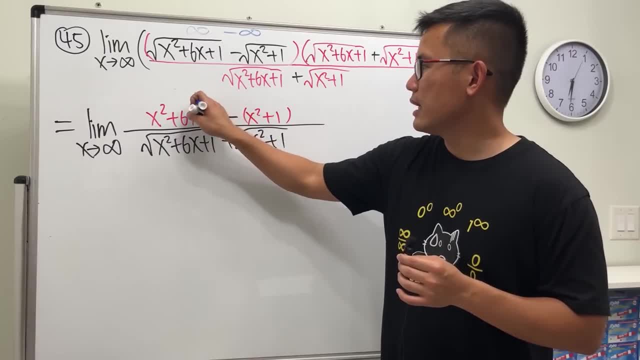 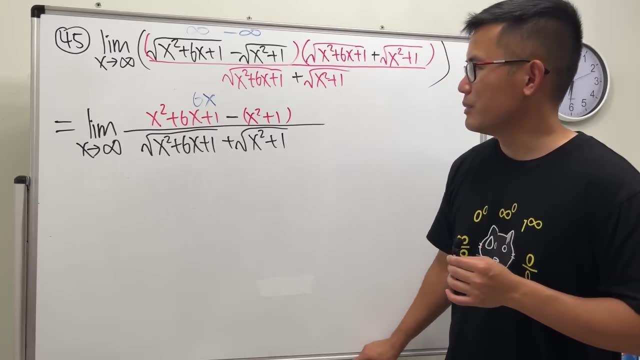 X squared, x squared, they cancel. We have six x on the top. Let me just put down the result here, And then one minus one. I think I'm just gonna rewrite everything again to make it super clear. So if we cancel the top, 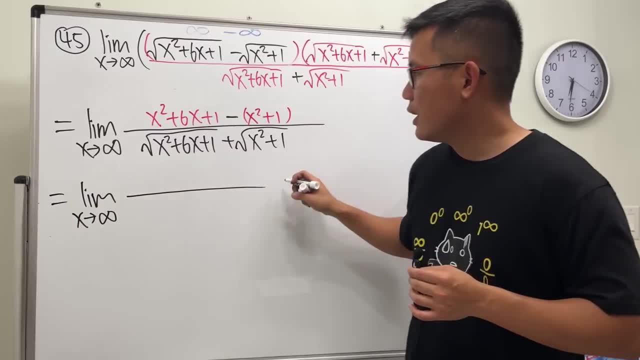 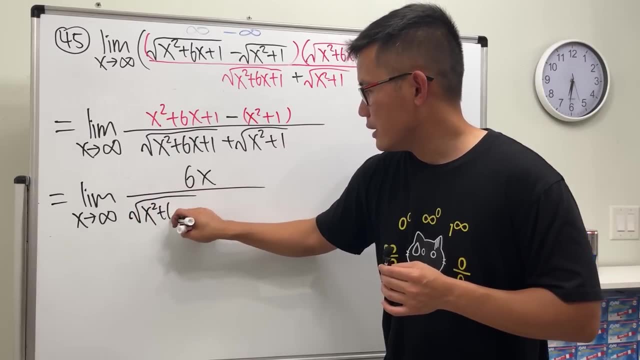 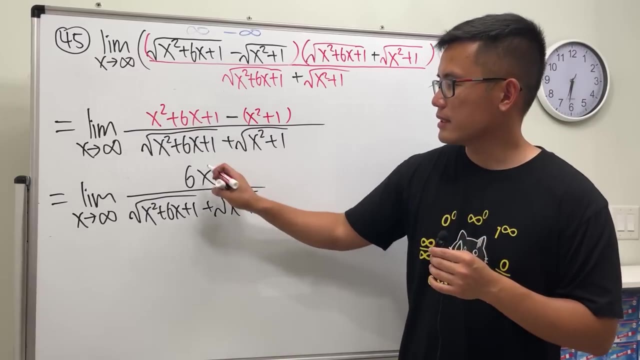 this is the limit. as x approaching infinity, We will just get six x on the top. One minus one is also gone, huh, And then all this, Okay, picked up the highest power of x on the top. It's just this six x to the first power. 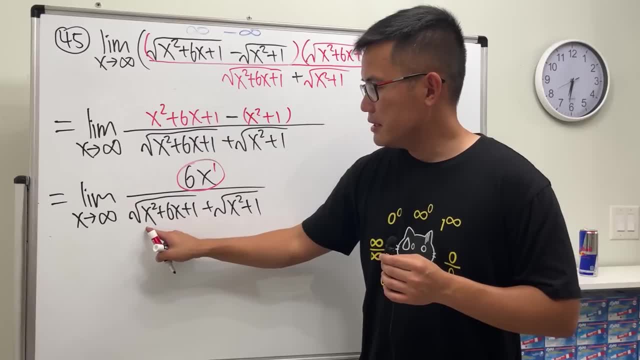 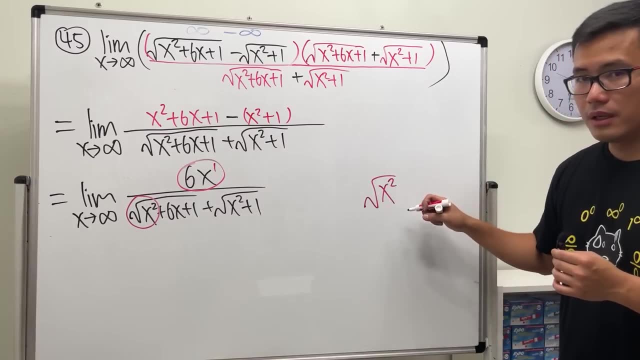 But guess what? On the bottom, this is the highest power, right here and square root of x squared. what's square root of x squared? Yes, we can cancel them, but if you just cancel them, you actually have to put an absolute value. 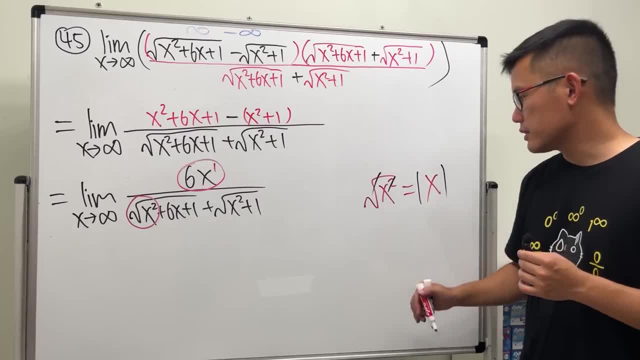 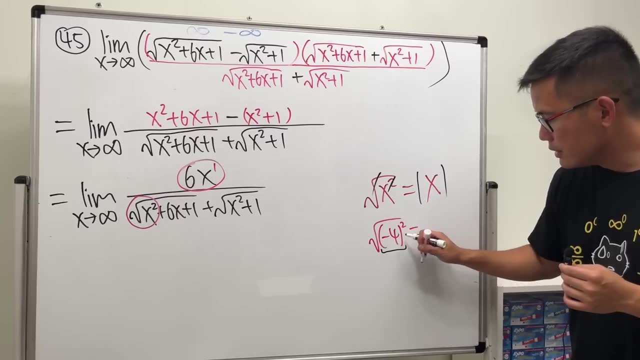 because the output of a square root is always positive. Quick example: when we have square root of negative, four squared. you do this inside out, this is 16, right, right and then take the square root, you get four. so you see if you have square root of negative. 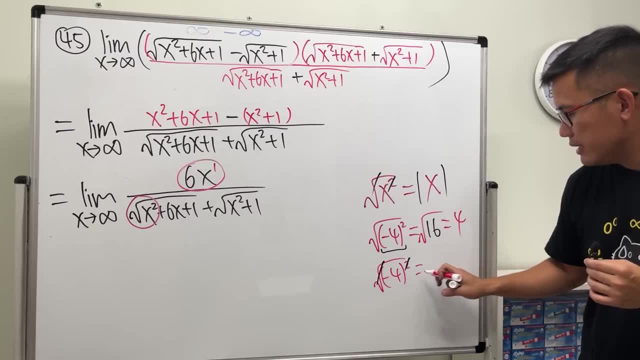 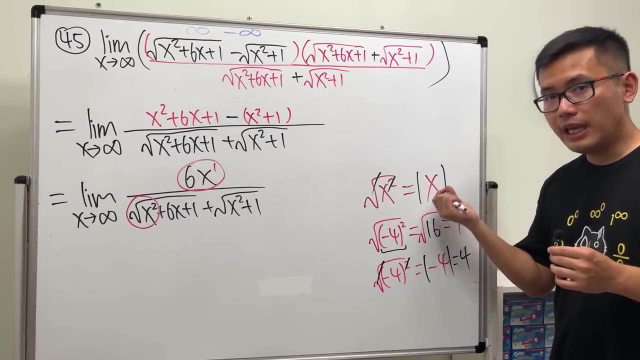 four square if you just cancel them and then just say the answer is negative four. this is wrong. you have to include the absolute value and then you see this is indeed equal to four. now okay. however, you don't need the absolute value if you know the inside, if you know the x is. 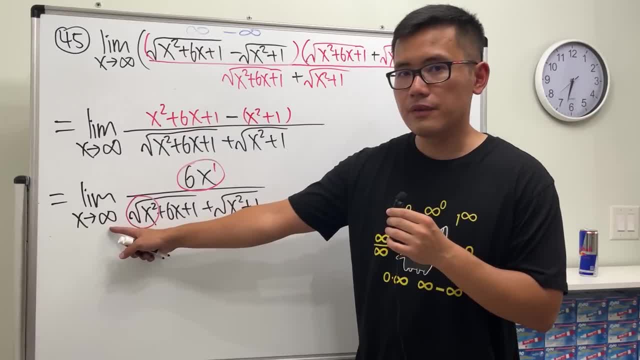 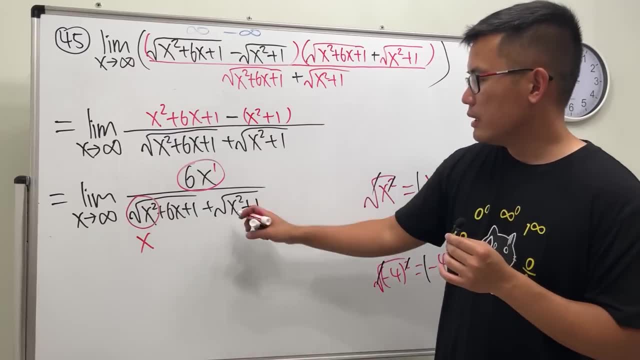 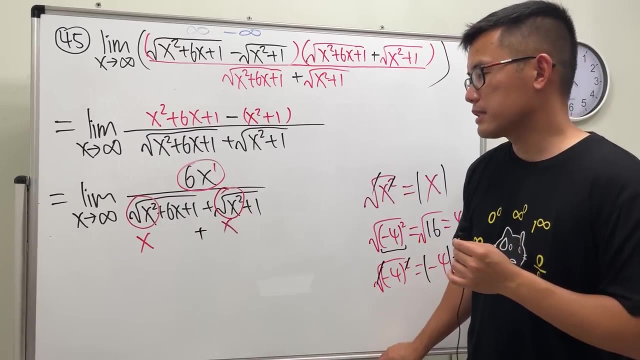 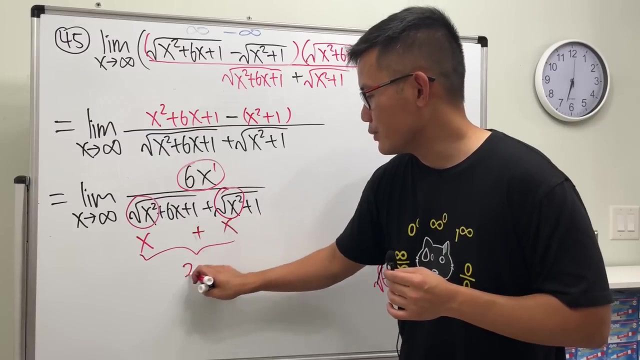 positive already. x is approaching positive infinity. so this part is just equal to x and that's legitimate, just x, no square root needed. likewise, here this is also equal to x. so guess what? on the bottom, we actually just have x plus x. wow, so technically, to get on the bottom, which is up to x, 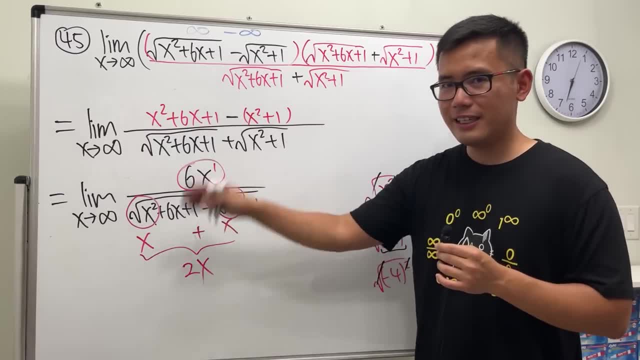 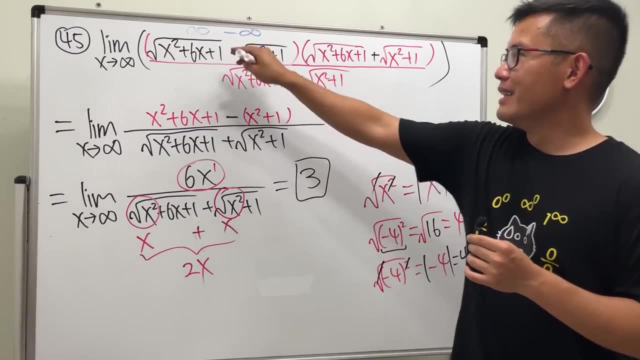 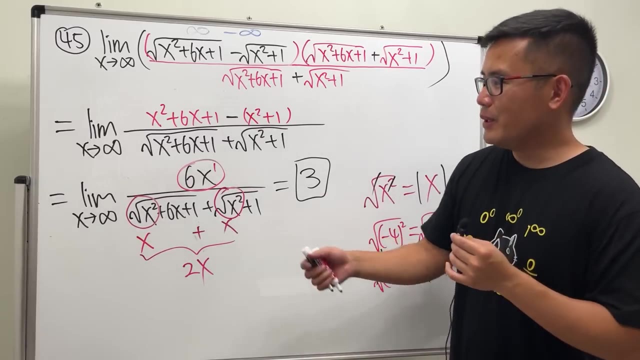 so 6x over 2x, dx cancel 6 over 2x. the answer is 3. ladies and gentlemen, i told you infinity minus infinity. hey, we also get a nice number three. can you get pi? yeah, if you manufacture a good example, yeah, you can get pi. 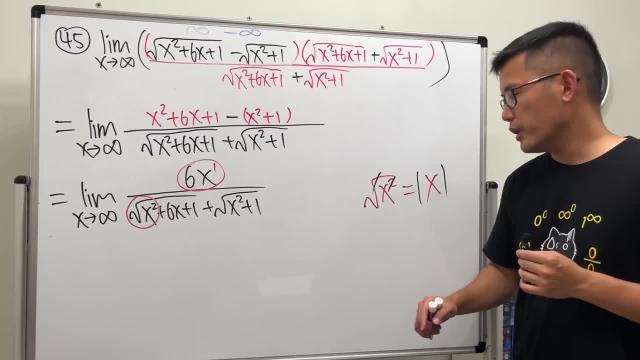 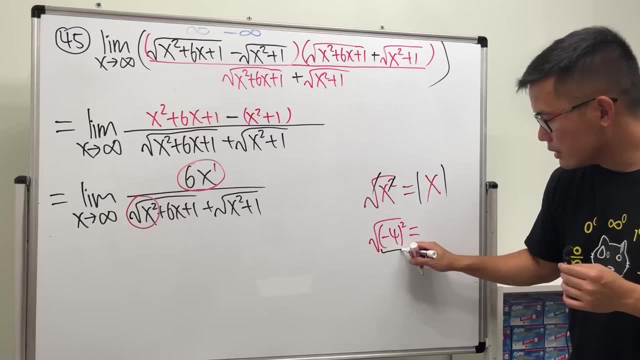 Because the output of a square root is always positive. Quick example: When we have square root of negative 4 squared, you do this inside out: This is 16,, right, And then take the square root, you get 4.. So you see, if you have 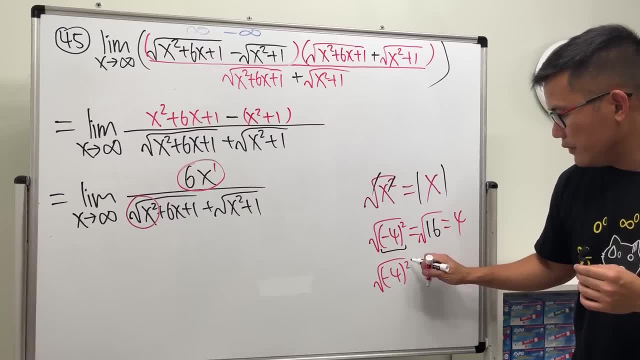 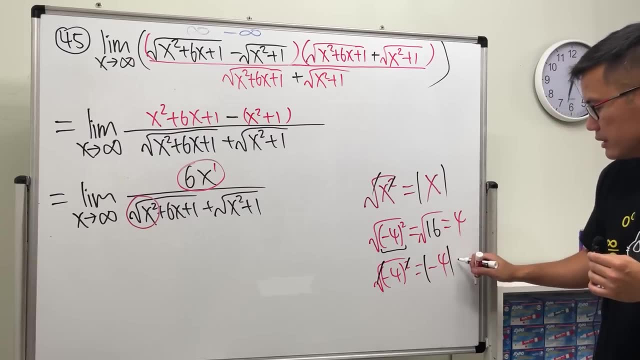 square root of negative 4 squared. if you just cancel them and then you just say the answer is negative 4, this is wrong. You have to include the absolute value And then you see this is indeed equal to 4 now. 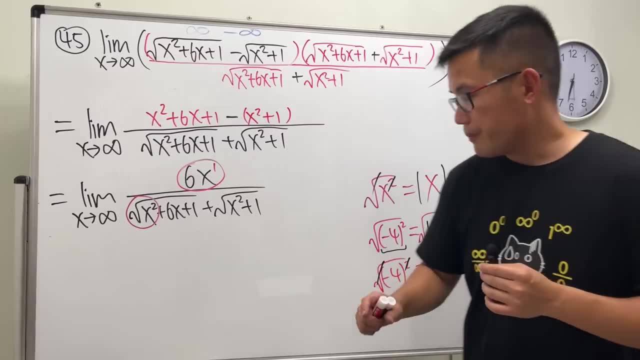 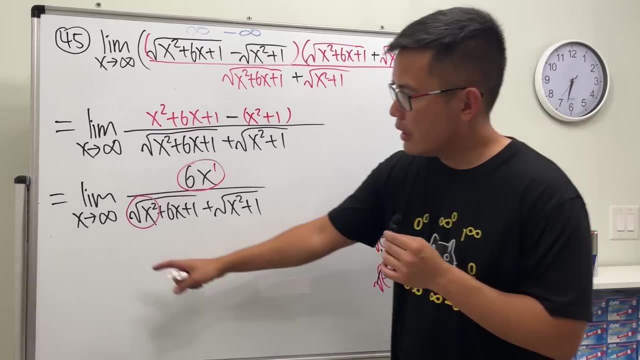 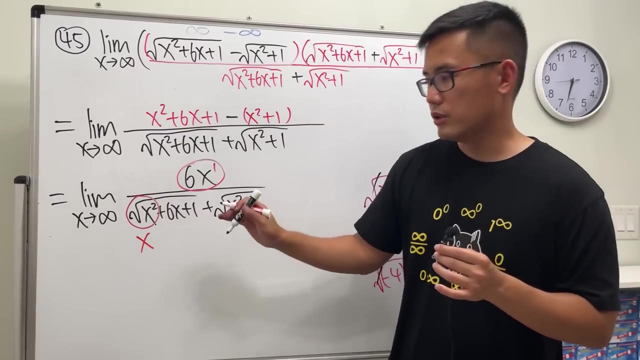 Okay. However, you don't need the absolute value if you know the inside, if you know the x is positive already x is approaching positive infinity. So this part is just equal to x and that's legitimate, Just x, no square root needed. 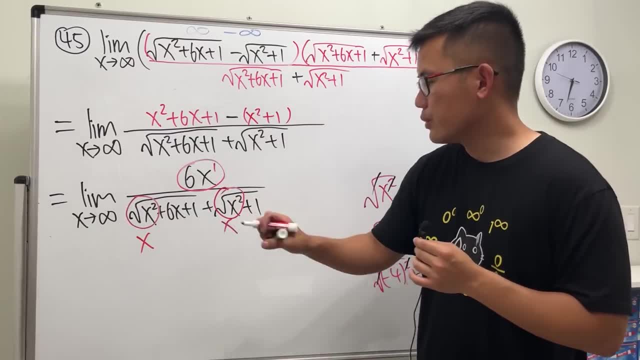 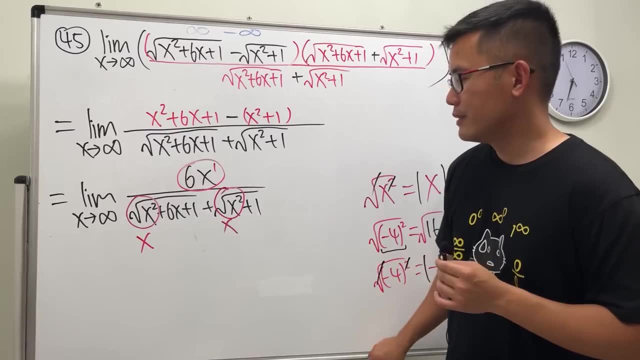 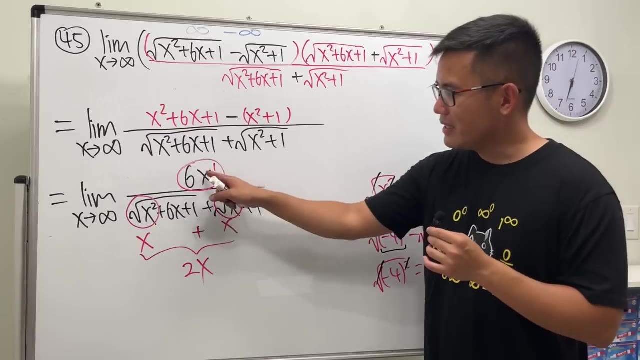 Likewise here. this is also equal to x. So guess what? On the bottom, we actually just have x plus 1. x- Wow. So technically, to get down the bottom, we just have 2x, So 6x. 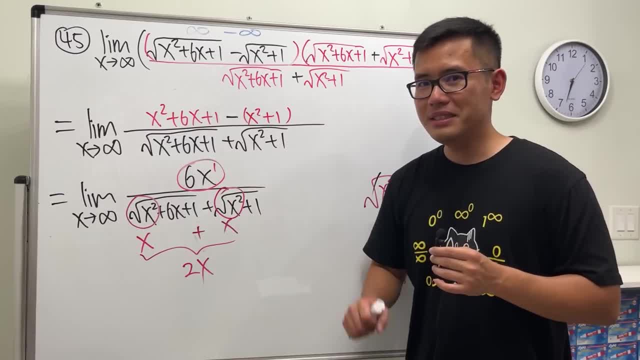 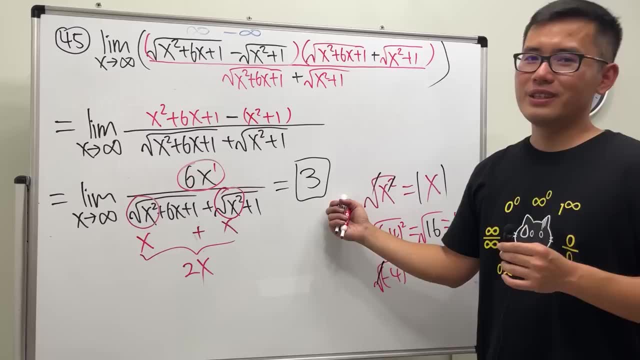 over 2x. the x cancel 6 over 2,. the answer is 3.. Ladies and gentlemen, I told you Infinity minus infinity. hey, we also get a nice number 3.. Can you get pi? Yeah, if you manufacture a good example. 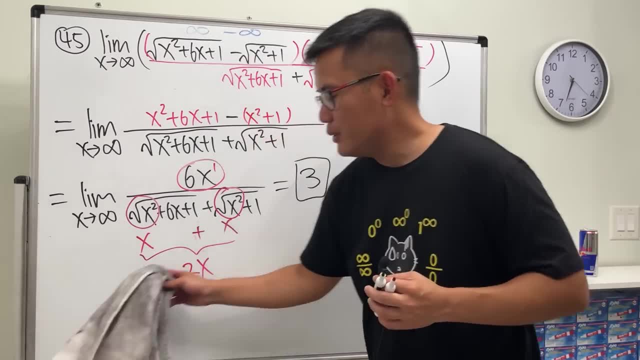 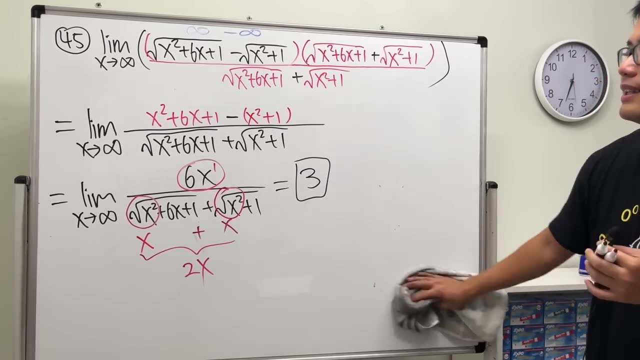 yeah, you can get pi. Can you get e to the 7th, 17 power minus 2.. Yeah, if you would like to try it, manufacture an equation it's possible. But again, infinity minus infinity it's not always equal to 0.. 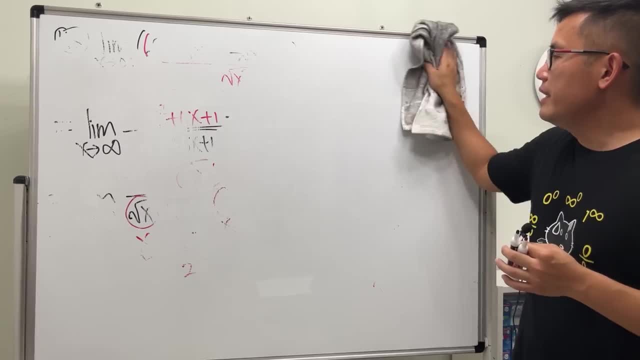 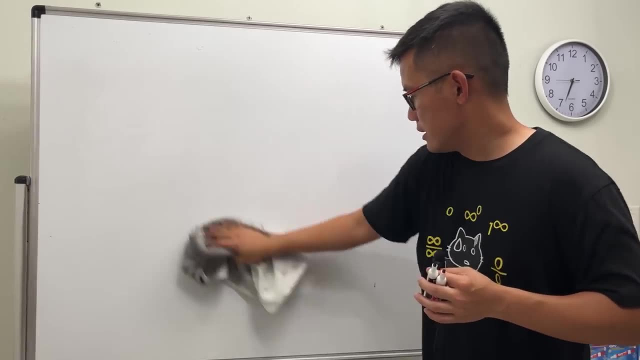 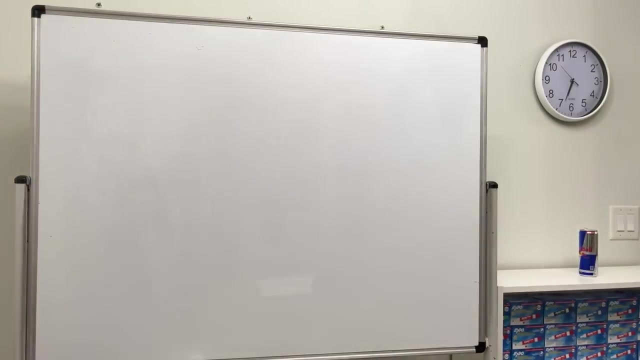 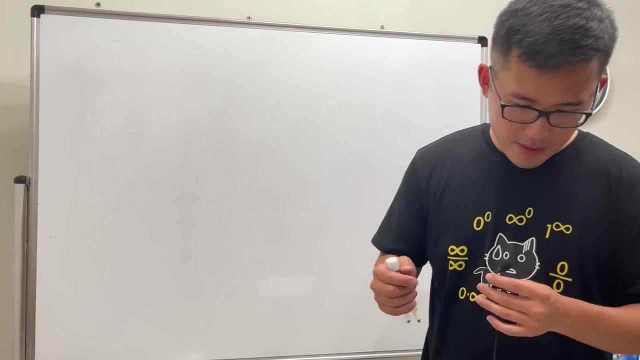 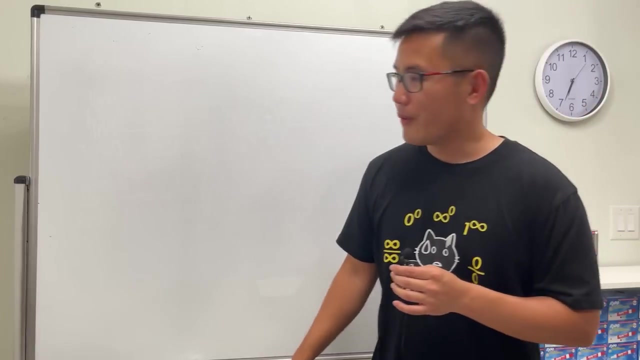 We cannot draw any conclusion unless we do more work, because that is an indeterminant form. Alright, number 45.. Let's take a look at- Wow, it's 3 hours already- Definition of derivatives. So I wanted to tell you guys. 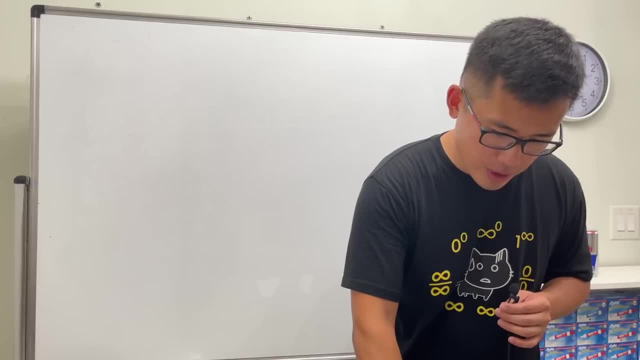 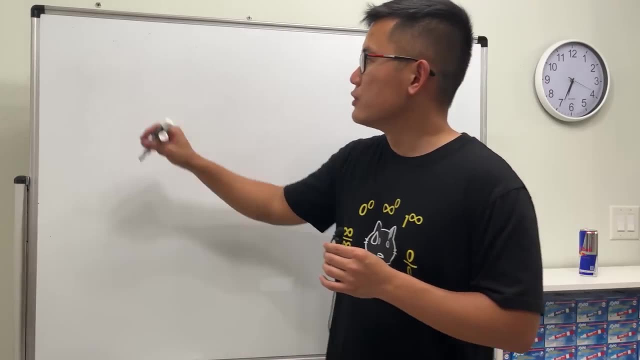 that for number 45, sorry for number 46- to number 50, we'll use the definition of derivative to calculate the derivative of a function as some number. So I will write this down for you guys: If we have f, prime of a, 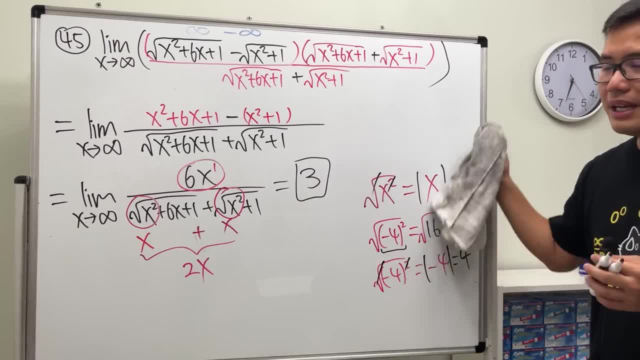 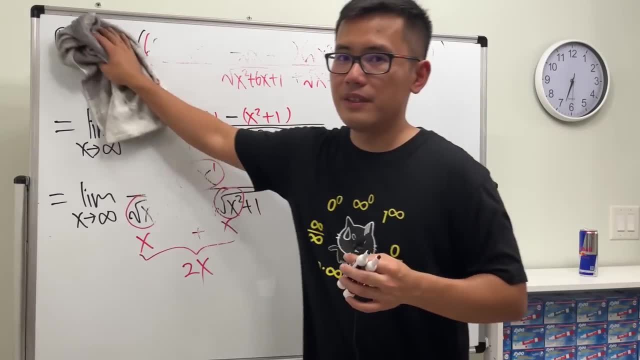 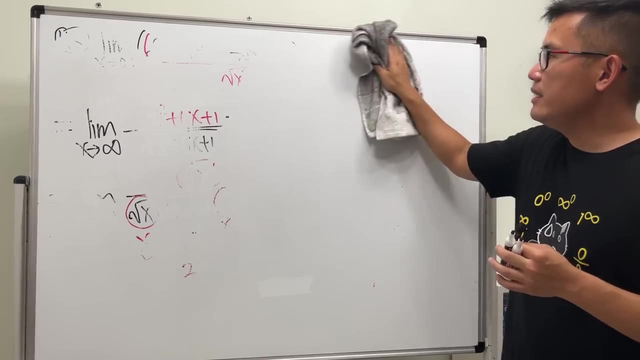 can you get e to the 17 power minus 2? yeah, if you would like, you can try it, manufacture a question, it's possible. but again, infinity minus infinity it's not always equal to zero. we cannot draw any conclusion unless we do more work, because that is an indeterminant form. 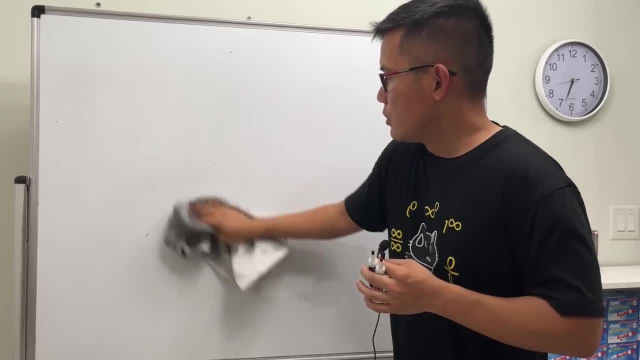 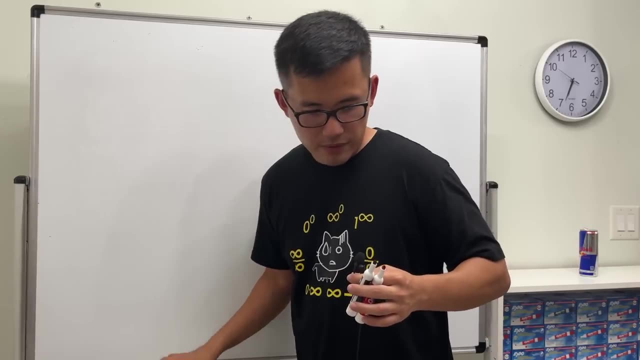 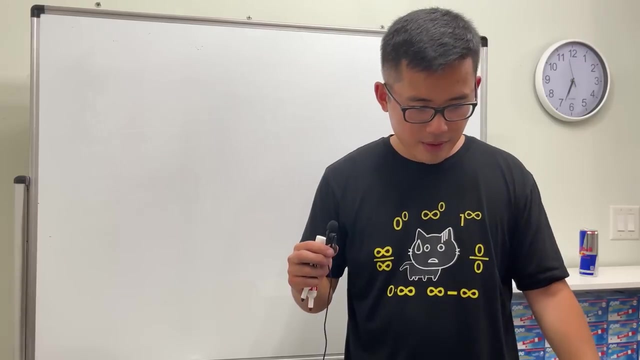 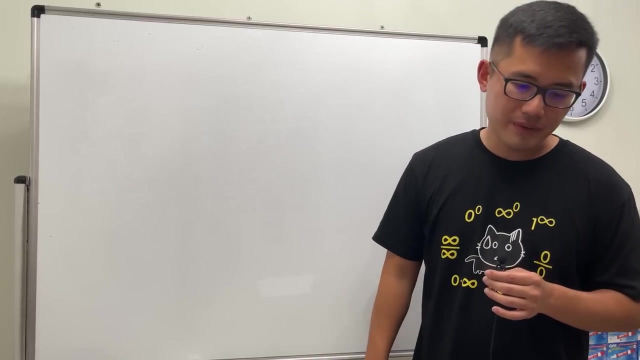 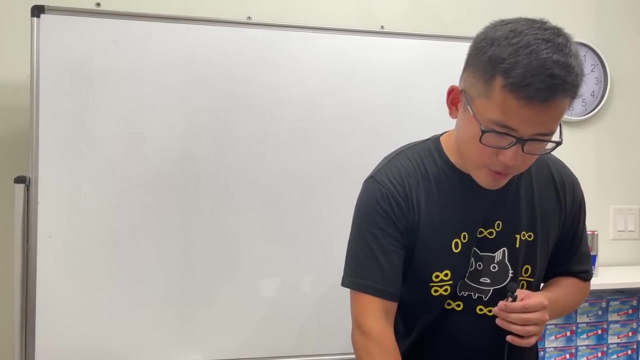 all right, number 45. let me just take a look at- uh wow, three hours already- definition of derivatives. so i wanted to tell you guys that for number 45- sorry for number 46 to number 50- we'll use the definition of derivative to calculate the derivative of a function. 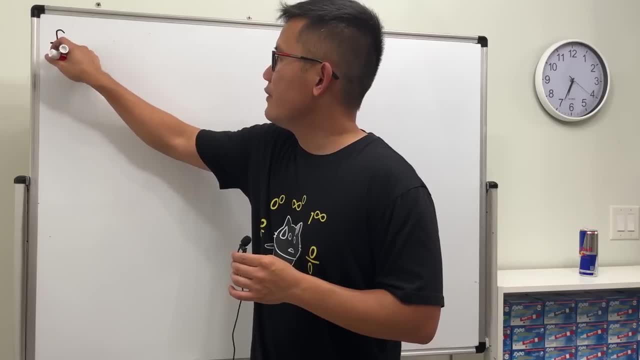 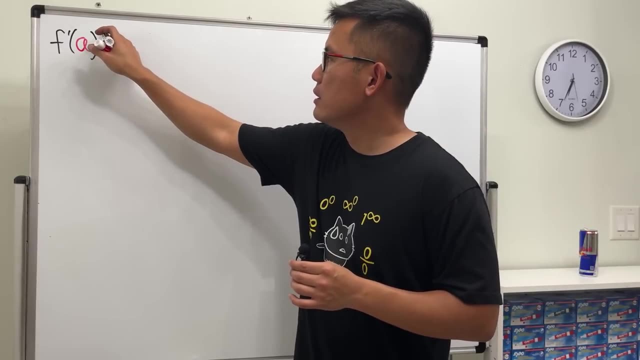 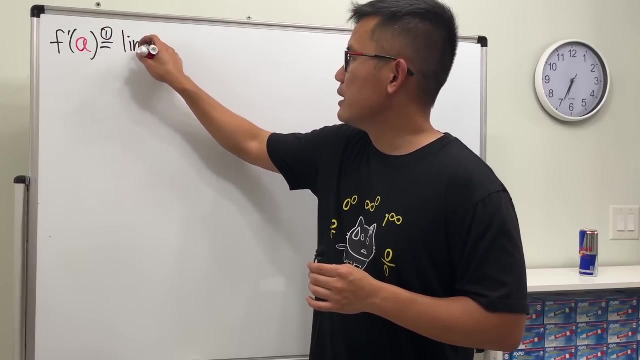 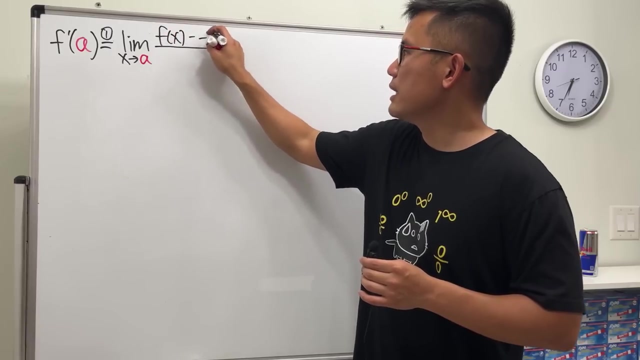 as some number. so i will write this down for you guys. if we have f prime of a, this right here i call this definition one. i'm just going to write it like this. yeah, so i call this definition one. this right here is the limit as x approaching a, and then we have f of x minus f of a. 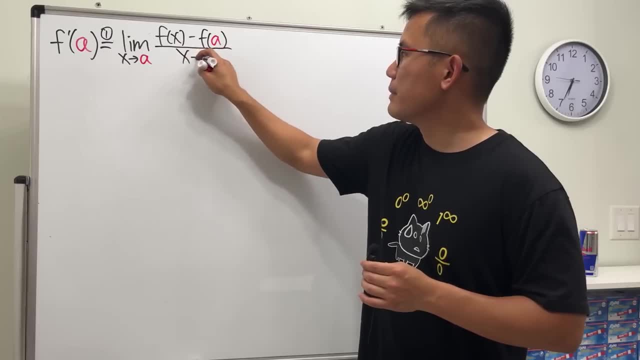 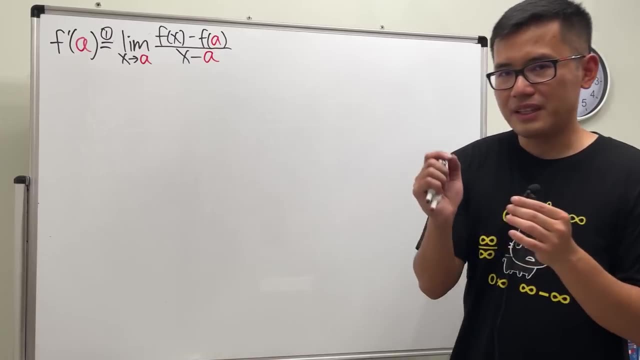 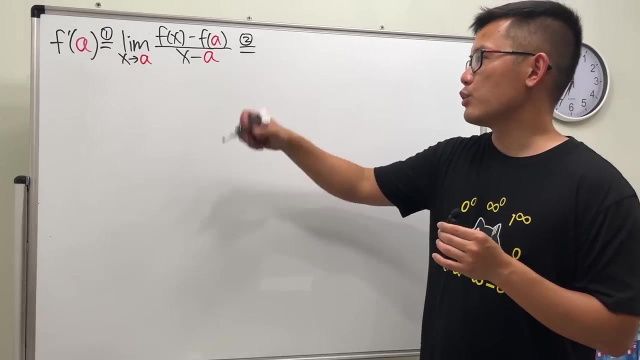 over x minus a. all right, so it's pretty much the difference of quotient. and then you let x approaching a. so that's how you can find the slope of the tangent line. secondly, this is what i call the definition of two. they are equivalent. this is the definition of two, and then you let x approaching a. 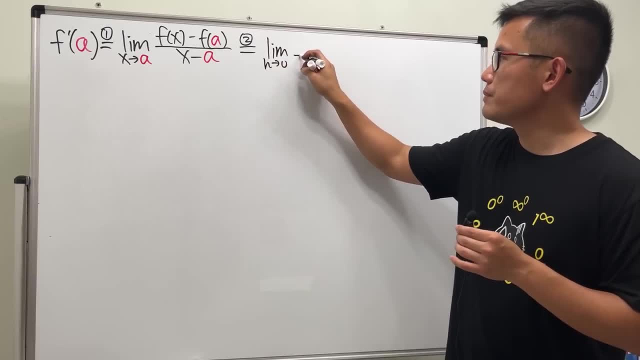 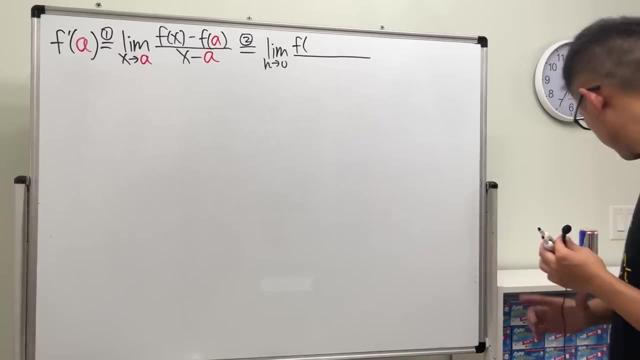 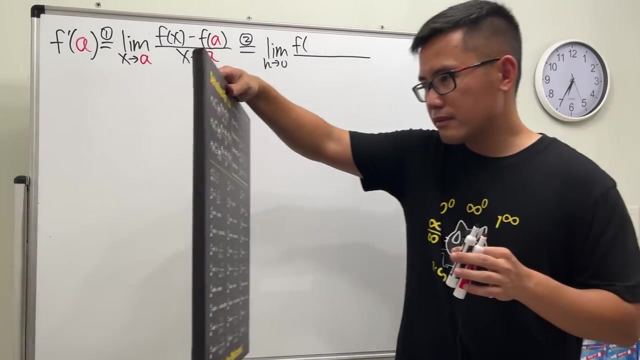 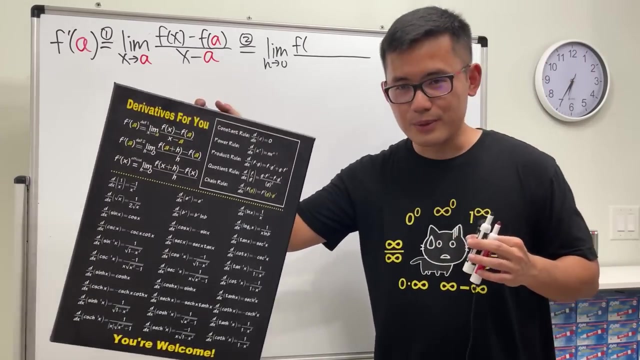 the one with H, the limit as H approaching 0.. And for this one we get f of. I forgot. Now I remember. Okay, I know My merge. Yeah, I designed this. I have a t-shirt and also a canvas print. 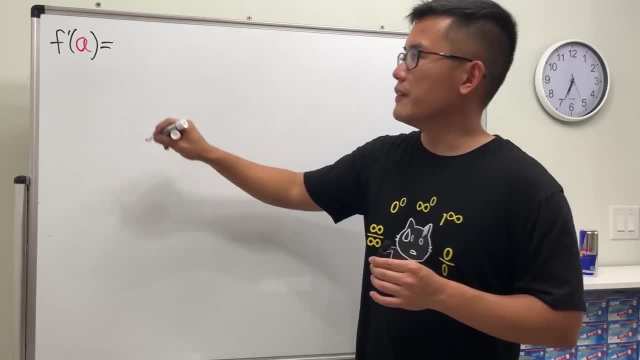 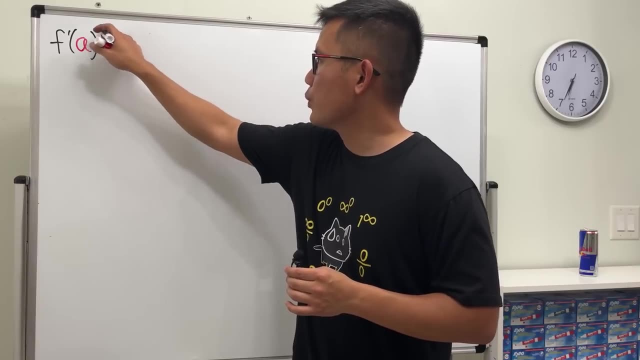 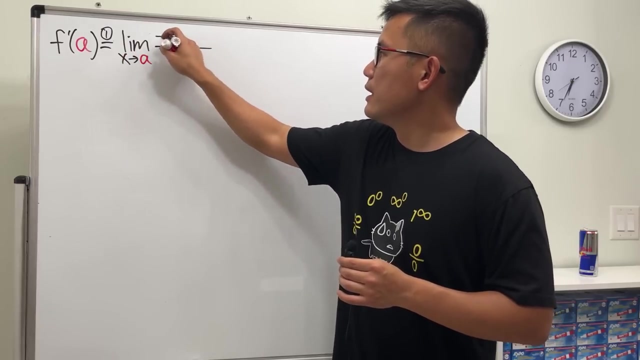 this right here. I call this definition 1.. I'm just going to write it like this, So I call this definition 1.. This right here is the limit as x approaching a, and then we have f of x minus f of a. 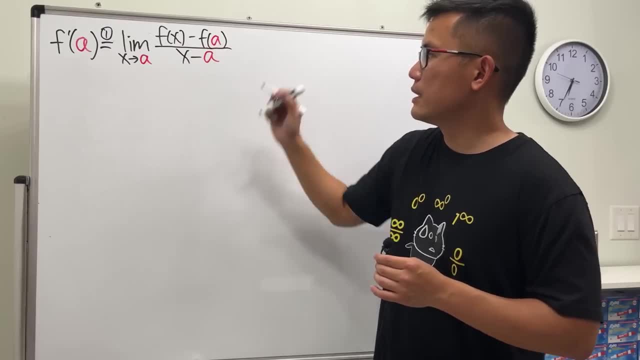 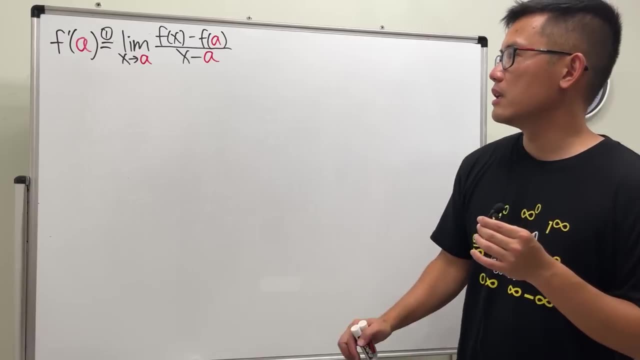 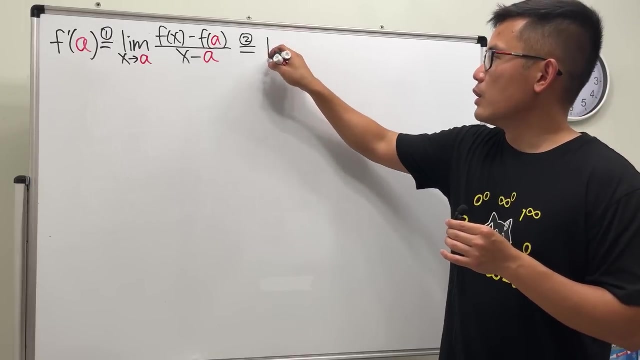 over x minus a. So it's pretty much the difference of quotient. And then you let x approaching a. So that's how you can find the slope of the tangent line. Secondly, this is what I call the definition of 2.. They are equivalent. 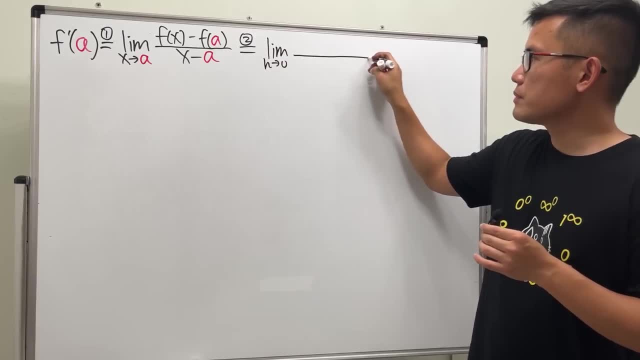 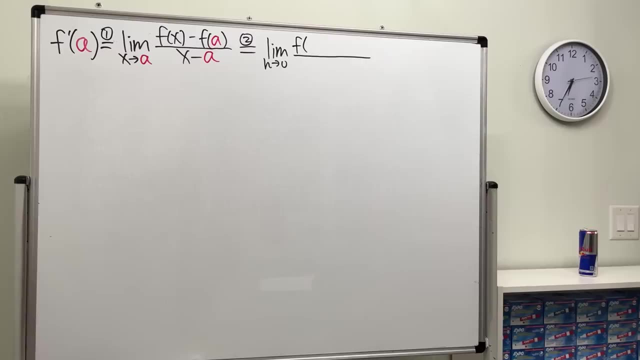 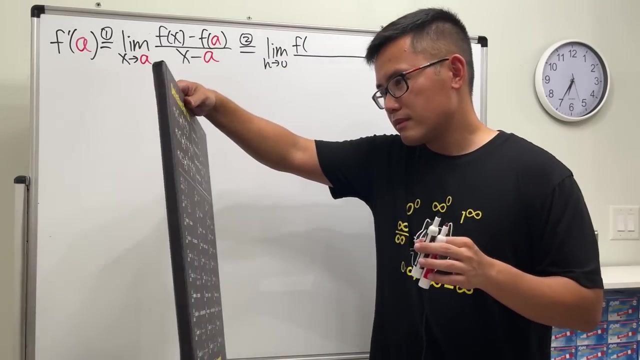 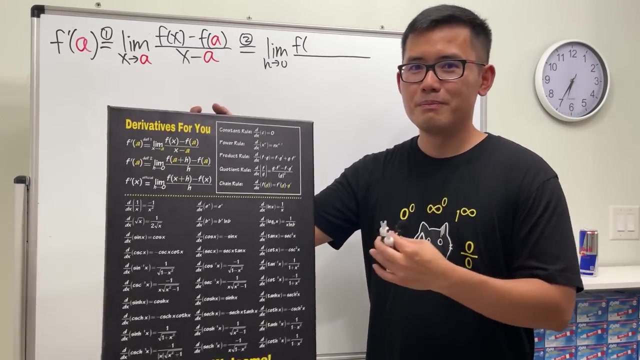 This is the one with h- The limit, as h approaching 0. And for this one we get f of I forgot Now, I remember, Now I remember, Now I remember. Okay, I know My merge. Yeah, I designed this. 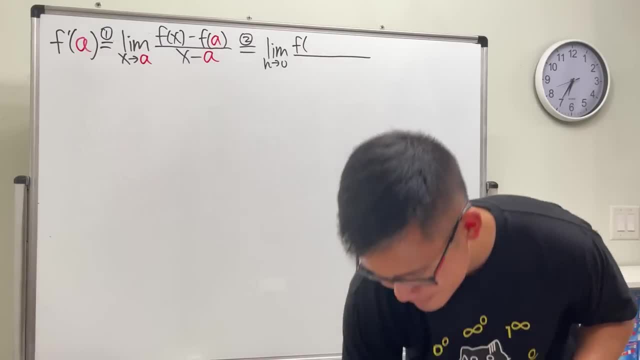 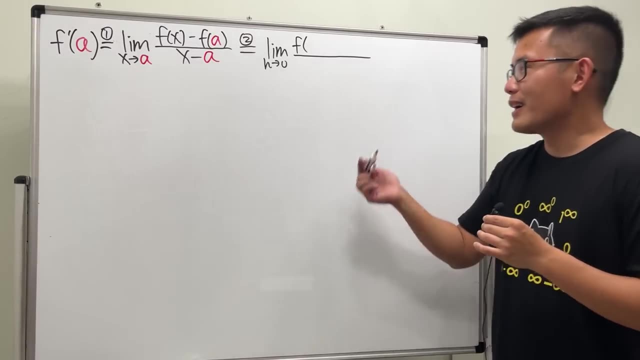 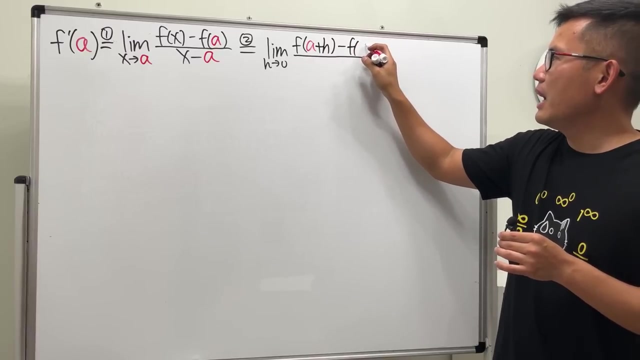 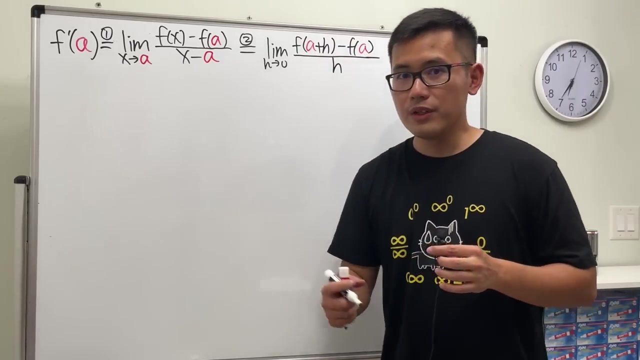 I have a t-shirt and also a canvas print Yeah, So I'll put it on the side. Okay, Alright, anyway, f of a plus h minus f of a. yeah over h. Okay. So definition 1, definition 2.. 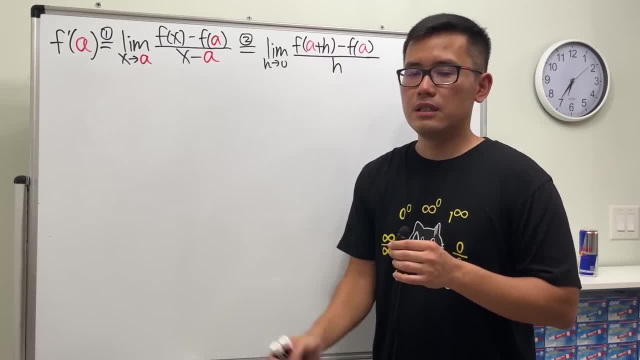 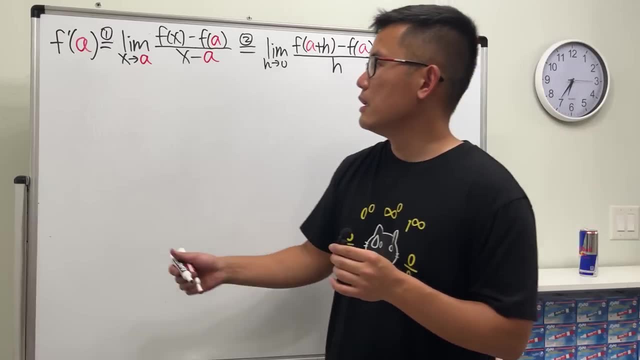 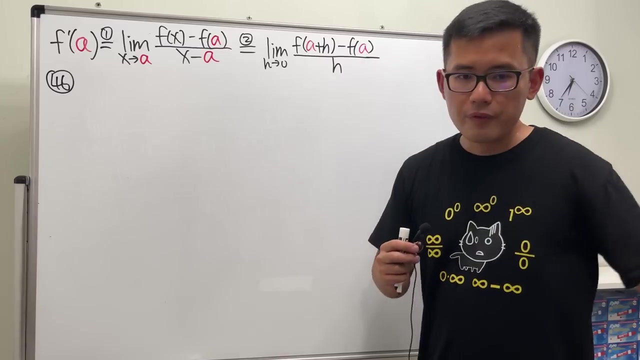 Let me just talk about them briefly. This right here is easier, if you like. factoring. This right here is easier, if you like. expanding. This right here is easier, if you like expanding. I have another video that I kind of compare both definitions. 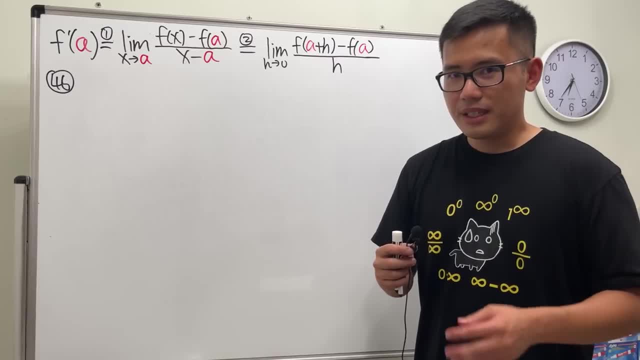 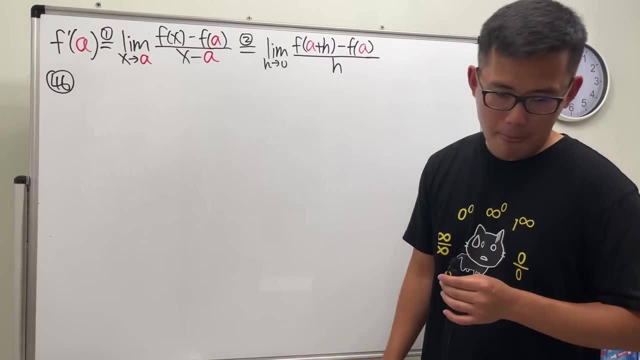 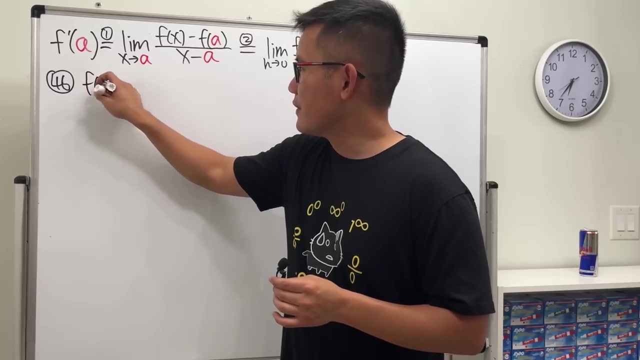 So you guys can take a look at that video. Take a look at that video, Not the channel, just calculus. Anyway, What are we doing? Okay, number 46. Let's say our function f of x is equal to 4x to the third power. 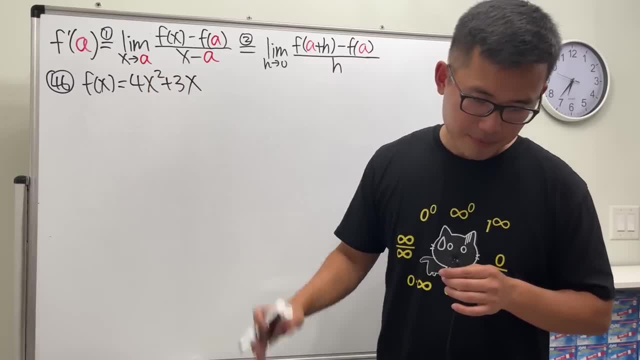 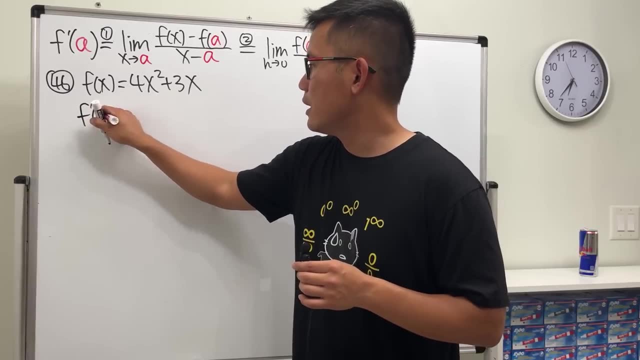 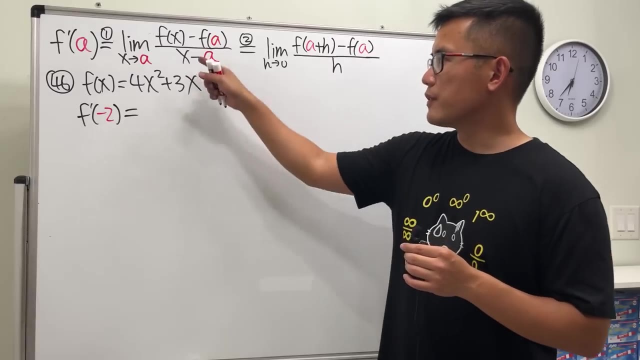 4x to the second power plus 3x. We want f of. we want f. prime of negative 2.. Okay, ladies and gentlemen, Number 46.. f, prime of negative 2.. Let's use the first definition. This is just a limit as x approaching. 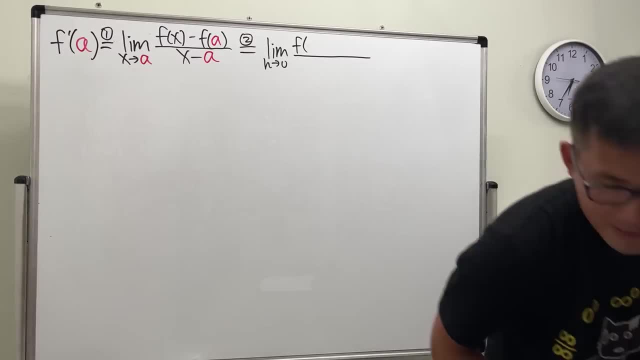 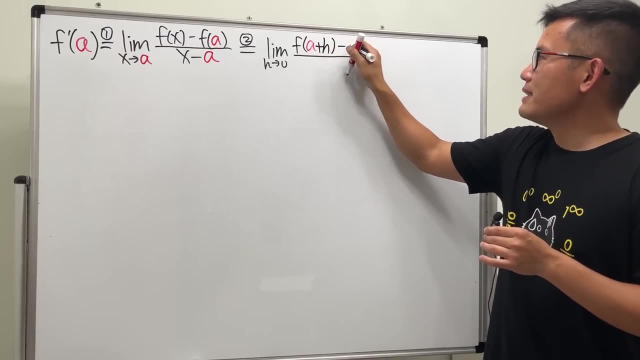 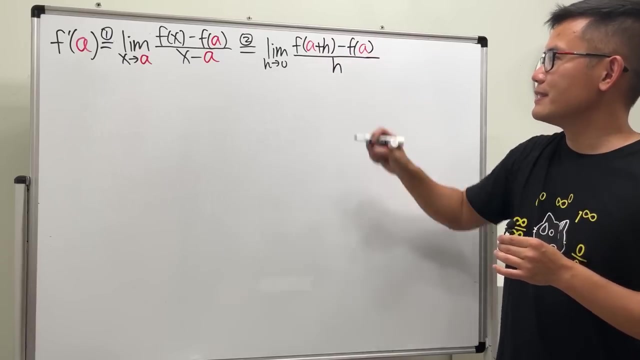 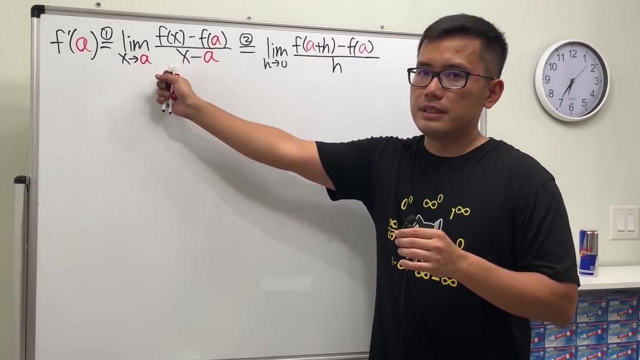 So I'll put it on the side. Okay, All right. Anyway, f of A plus H minus f of A, yeah, over H. Okay, So definition one, definition two. Let me just talk about them briefly. This right here, it's easier, if you like, factoring. 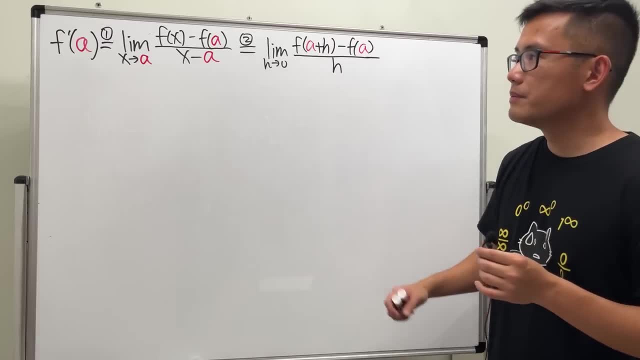 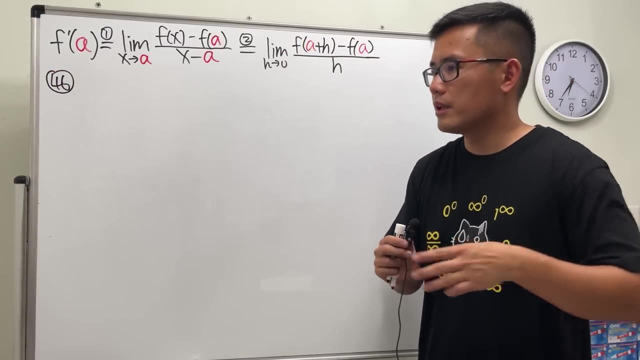 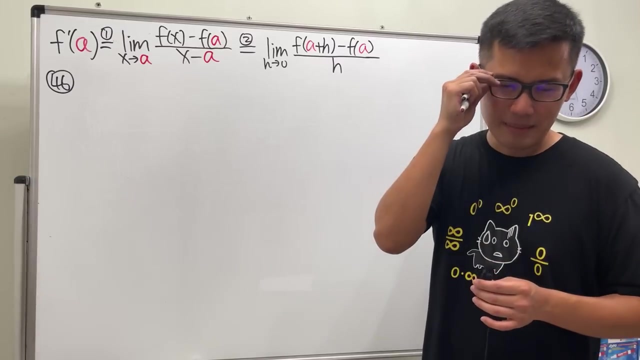 This right here. it's easier if you like expanding, So that's the advantage. And also I have another video that I kind of compare both definitions, So you guys can take a look at that video on my another channel, Just Calculus. 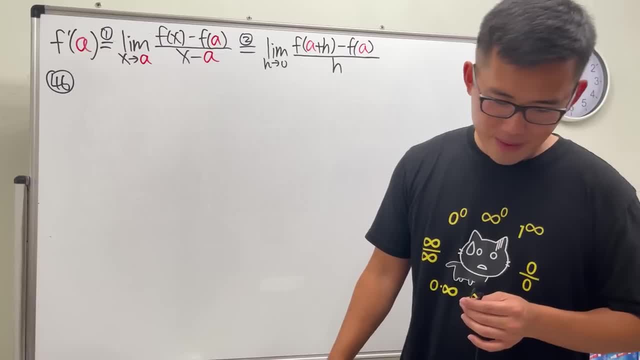 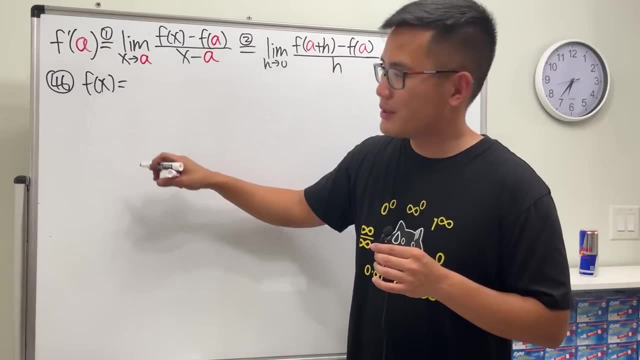 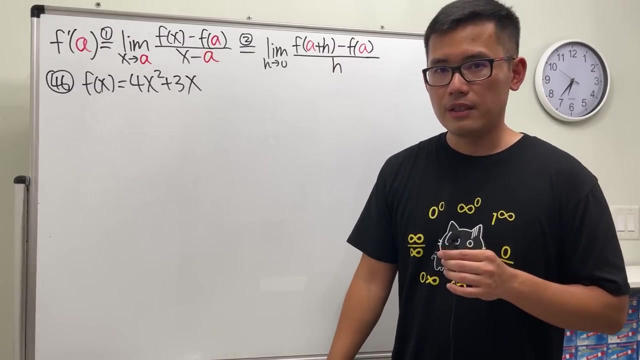 Anyway, what are we doing? Okay, number 46. Let's say our function f of x is equal to 4x to the third power, 4x to the second power plus 3x. We want f prime of negative two. 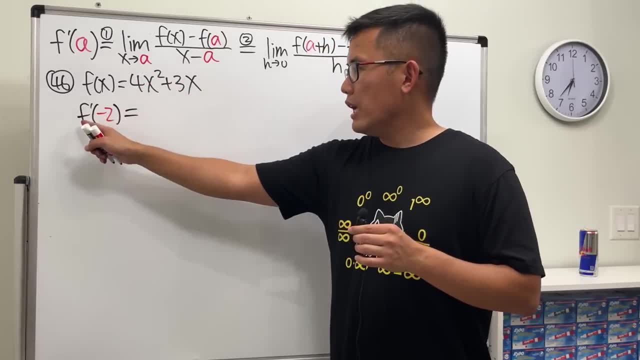 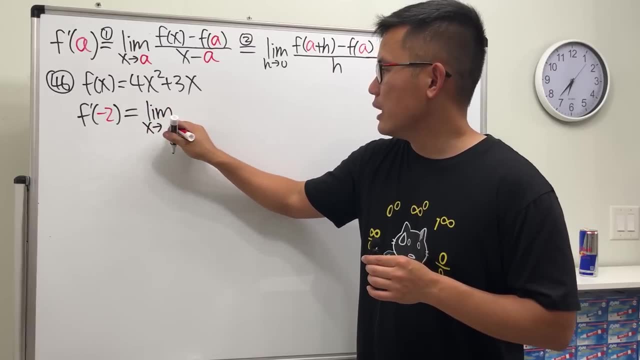 Okay, ladies and gentlemen, number 46, f- prime of negative two. Let's use the function f- prime of negative two. Let's use the function f- prime of negative two. Let's use the function f- prime of negative two. Let's use the first definition. This is just the limit as x approaching. 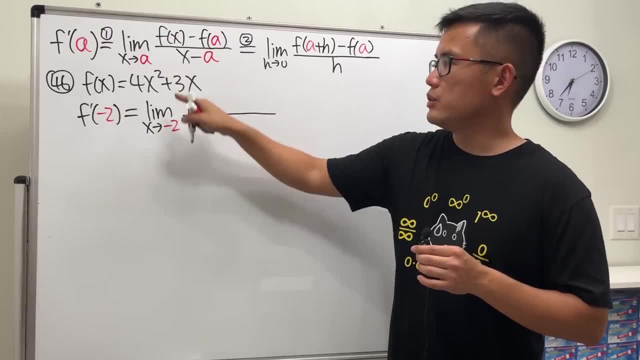 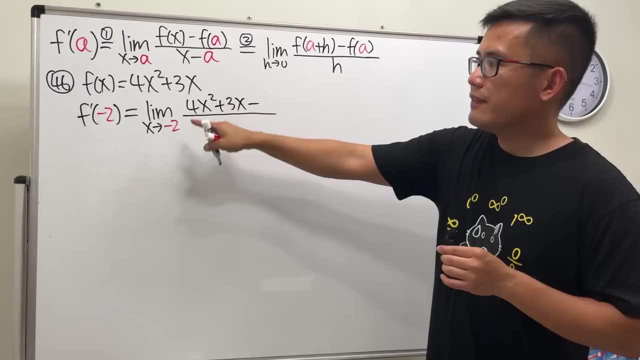 negative two And you see, f of x is just that. So we can just put that here: 4x squared plus 3x and then minus. we need f of negative two. So let's put it on the side. That's what I should do here. f of negative two. 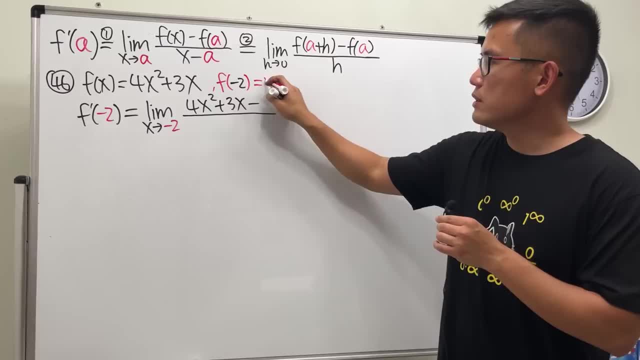 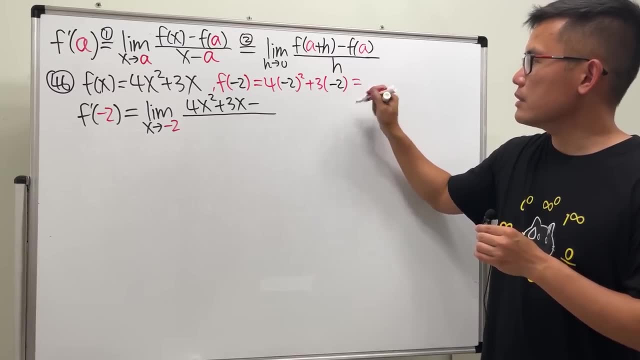 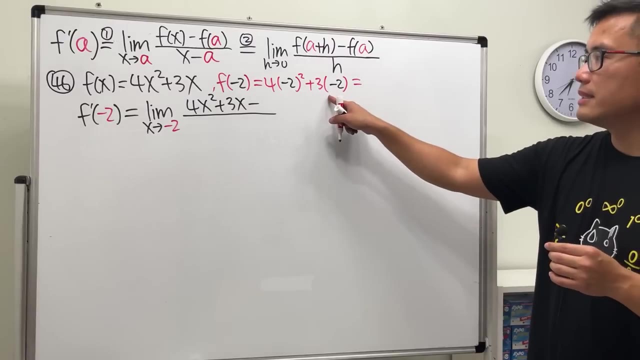 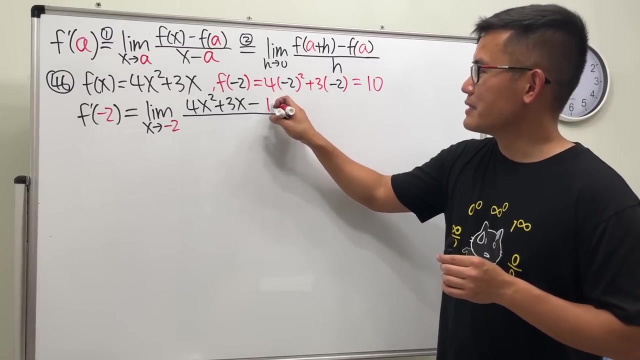 means we're plugging negative two into this x and that x, So we get four times negative two squared, plus three times negative two. This is four times that is 16.. Yes, 16 minus six is 10.. Yes, so this right here is minus 10.. So f of negative two is 10.. And then on the bottom, 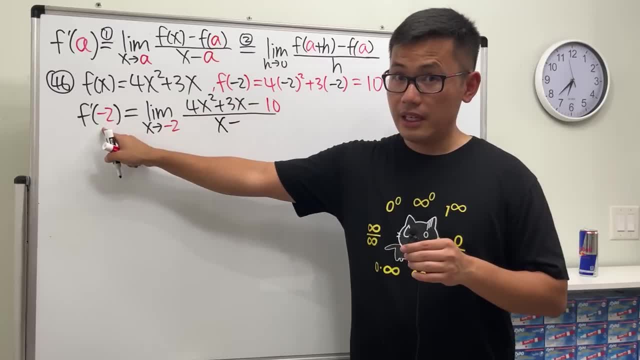 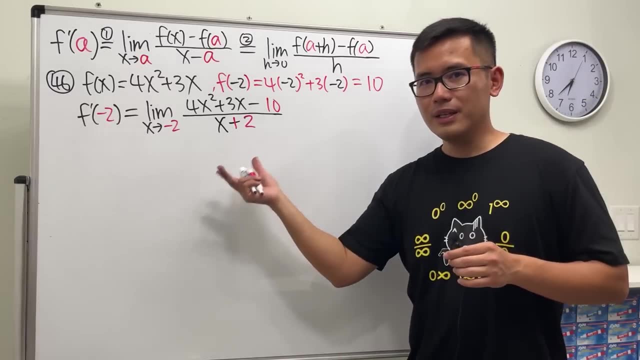 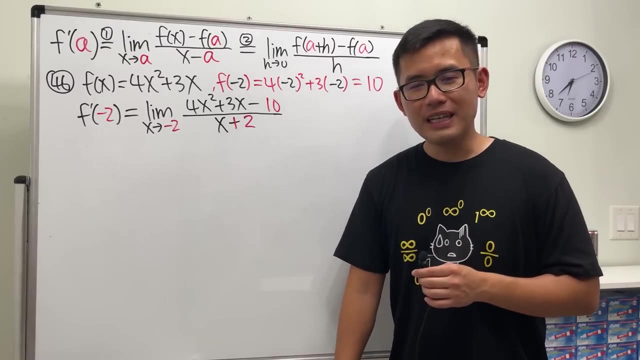 we have the x minus a is negative two, So minus minus becomes plus two. All right, cool. And now, if you take a look right here, doesn't this remind you of the algebraic limits that we did? Yes, Is there a fast way to do this? Yes, but let's do the things that we did. 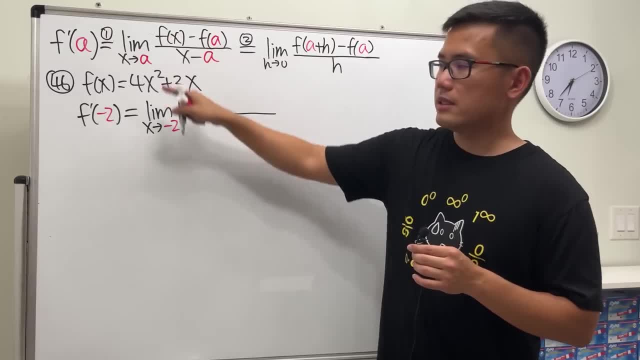 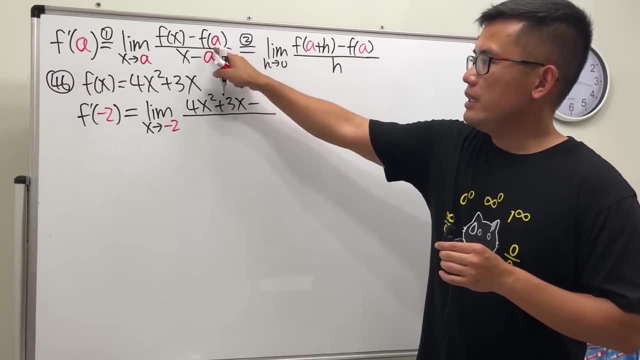 negative 2.. And you see, f of x is just that. So we can just put that here: 4x squared plus 4x and then minus. we need f of negative 2.. So let's put it on the side. That's what I should do here. 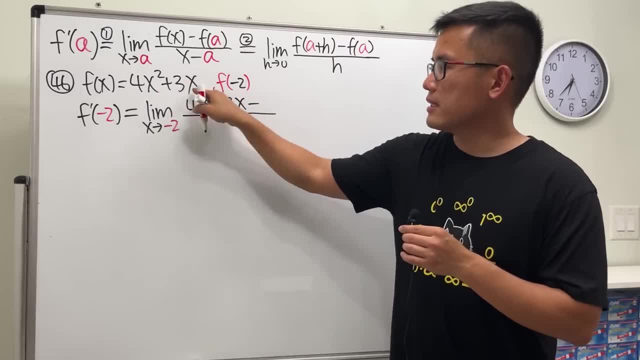 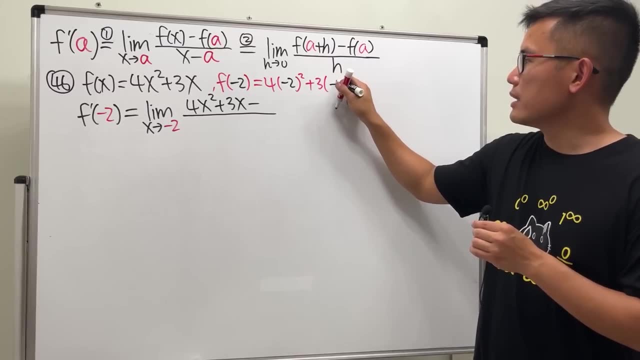 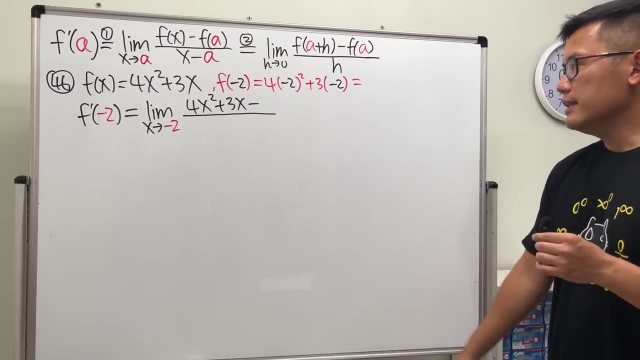 f of negative 2 means we're plugging negative 2 into this x and that x, So we get 4 times negative 2 squared, plus 3 times negative 2.. This is 4 times that is 16.. Yes, 16 minus 6. 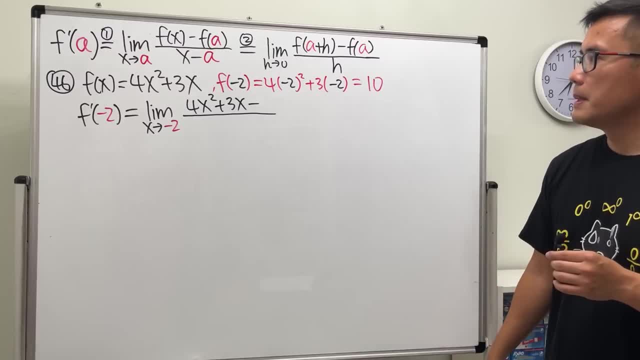 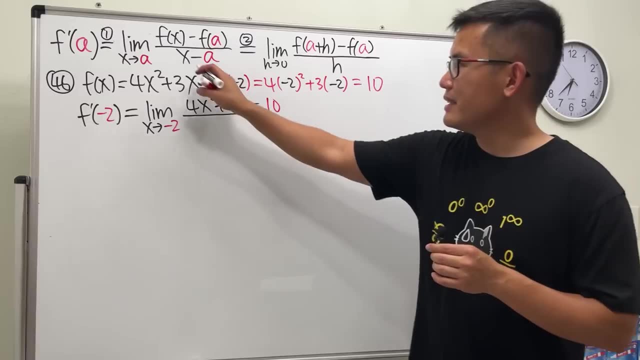 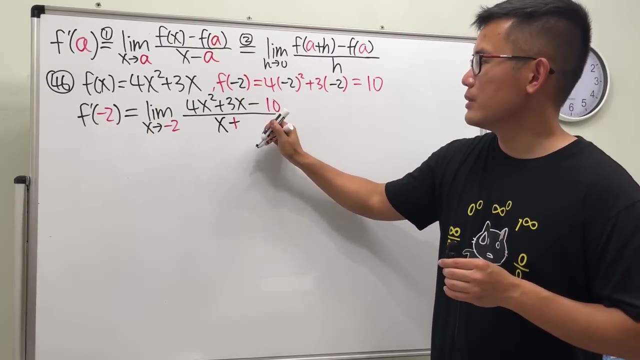 is 10.. Yes, So this right here is minus 10.. So f of negative 2 is 10.. And then on the bottom we have the x minus a is negative 2.. So minus minus becomes plus 2.. Alright, 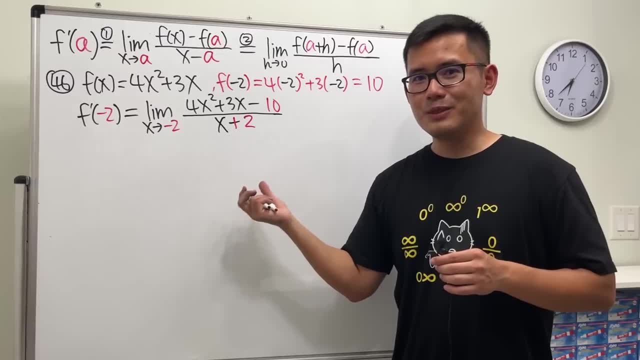 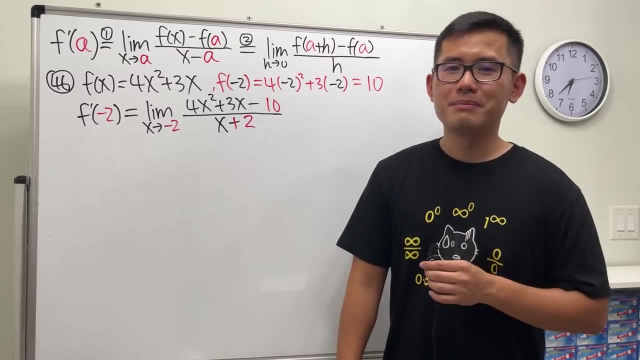 Cool. And now, if you take a look right here, doesn't this remind you of the algebraic limits that we did? Yes, Is there a fast way to do this? Yes, But let's do the things that we did earlier. Okay. 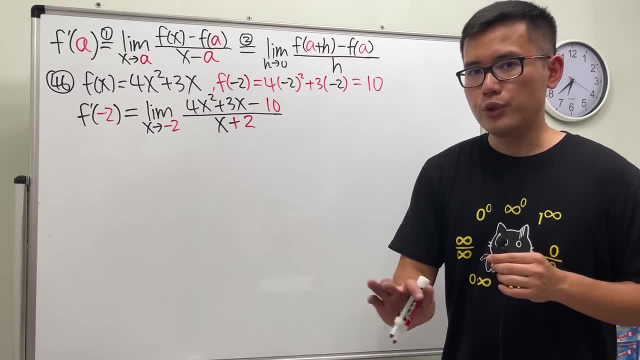 I'll tell you: If you put negative 2 into all the x's, for sure you get 0 for 0. Why? Because we set it out to be 0 for 0. When we put a into this x and that x, 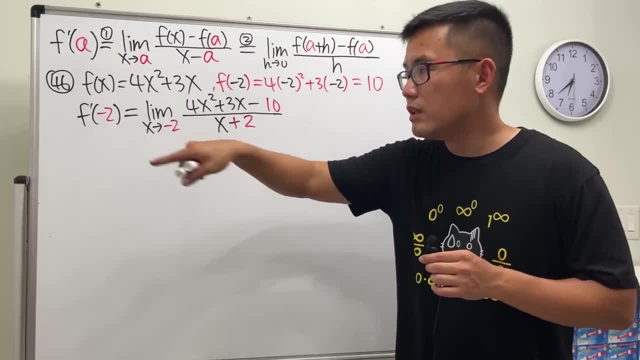 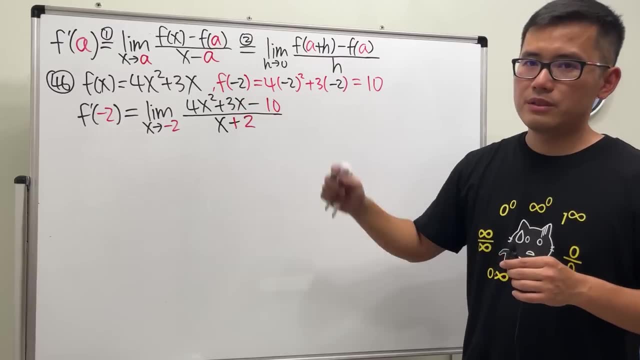 it was f of a minus f of a 0, a minus a 0. Likewise here, 0 for 0. If you don't get 0 for 0, then that means you set it out wrong. Anyway, though, how do we simplify? 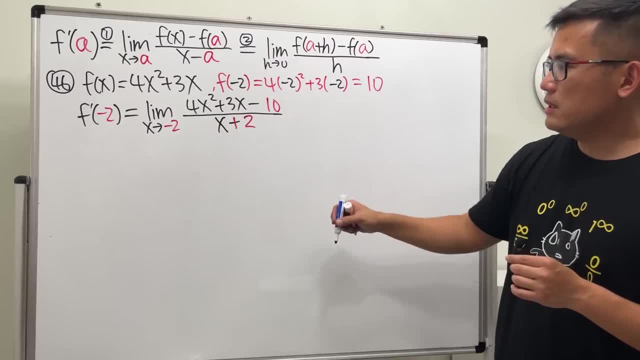 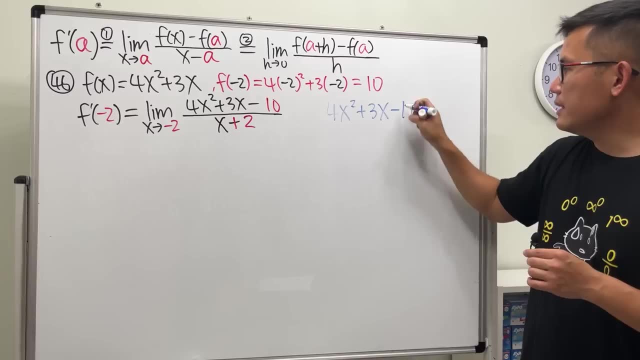 this. We can actually just factor it. So let me see, Let me put it down on the side: 4x squared plus 3x minus 10.. No common factor. so we'll just do a tic-tac-toe right away. 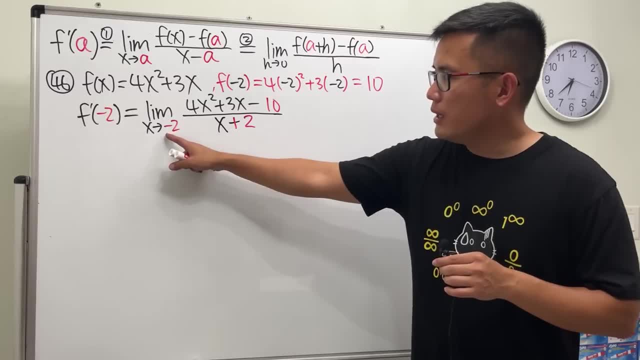 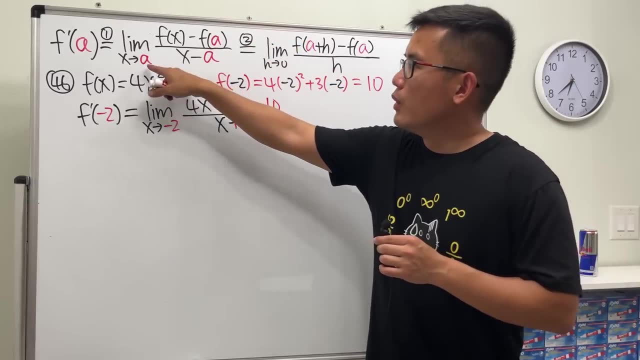 earlier. Okay, I'll tell you. if you put negative two into all the x's, for sure you get zero over zero. Why? Because we set it up to be zero over zero When we put a into this x and that x. 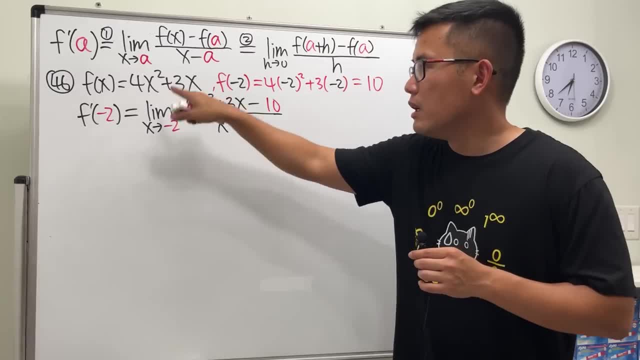 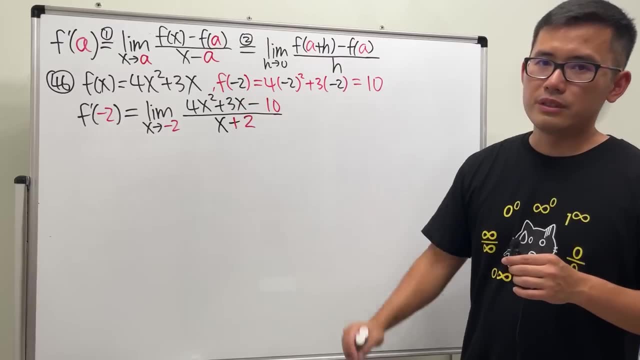 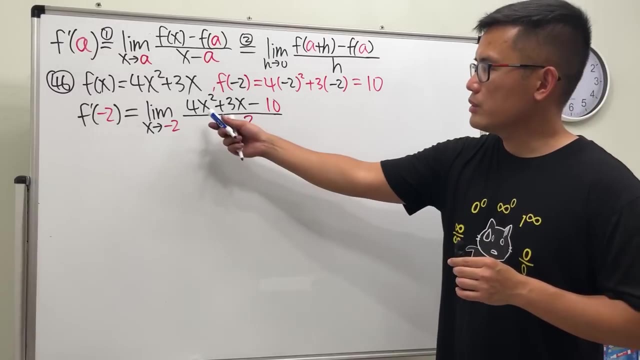 it was f of a minus f of a zero, A minus a zero. Likewise here: zero over zero. If you don't get zero over zero, then that means you set it up wrong. Anyway, though, how do we simplify this? We can actually just factor it. 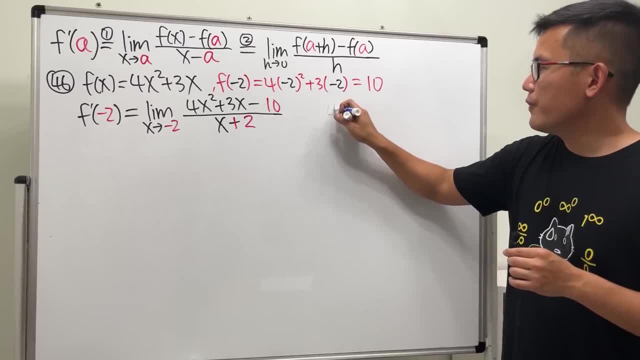 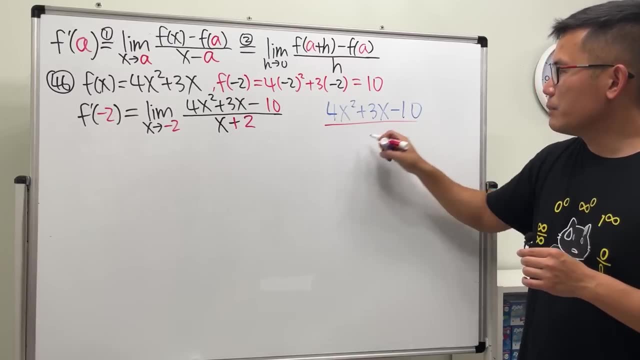 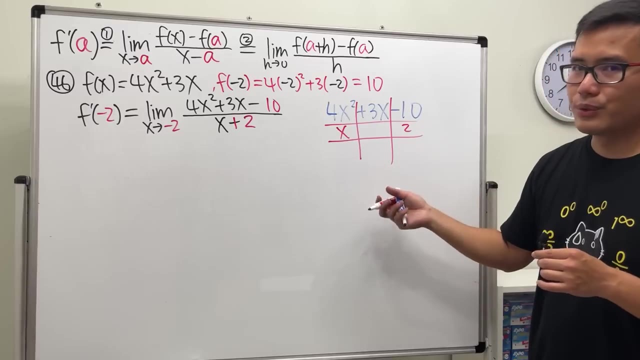 So let me see, Let me put it down on the side: Four x squared plus three x minus 10.. No common factor. so we'll just do a tic-tac-toe right away. So you know the deal. We need to have x and two right here. Four x two times four will be negative. 10 is negative five. 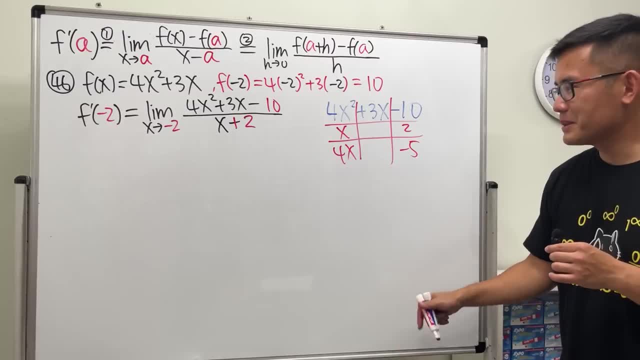 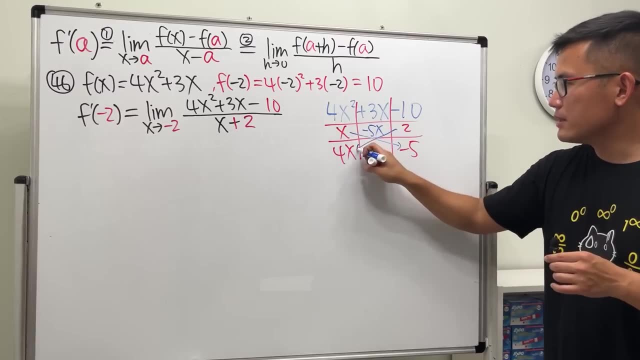 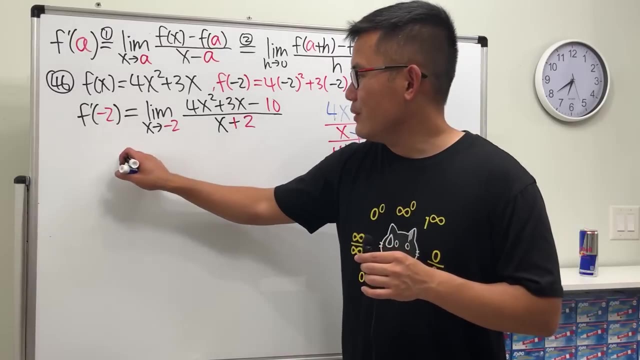 Why does this work? We need to get rid of that. All right, so that's it. But check this out: X times negative five is negative five x, and then two times four x is eight x. Together, we do get a three x that we want. Okay, so this is the limit as x approaching negative. 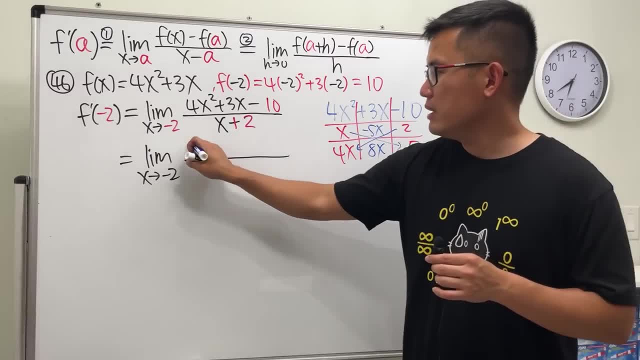 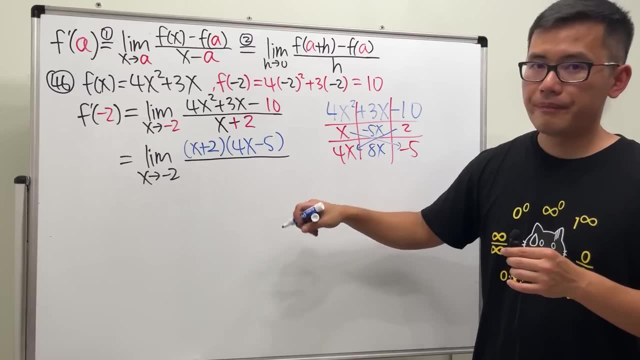 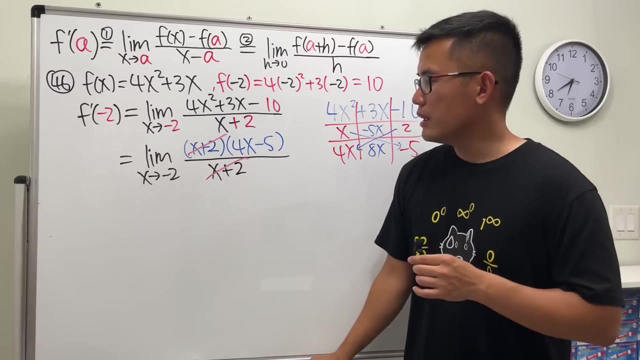 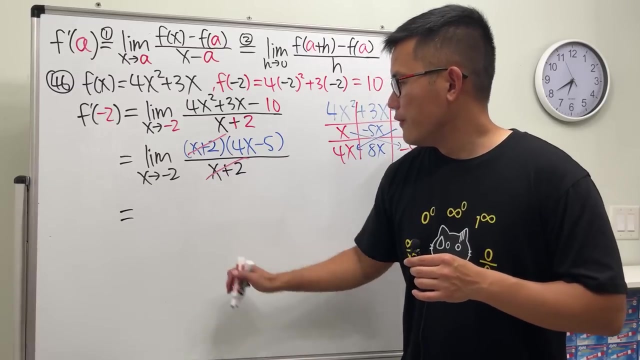 two On the top is just that, namely x minus, so x plus two times four, x minus five. On the bottom, it's still x plus two. Overall, though you see that this and that can cancel, Finally, put a negative two into here and we will get four times negative two and then minus five. 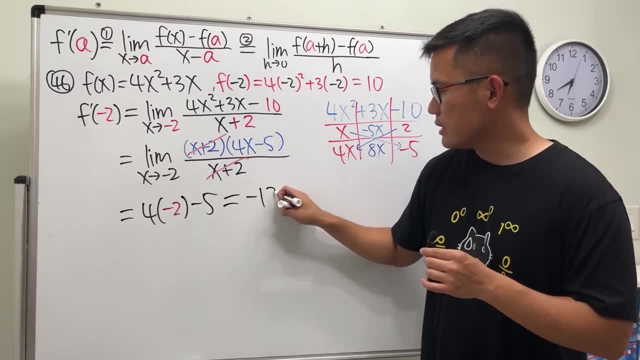 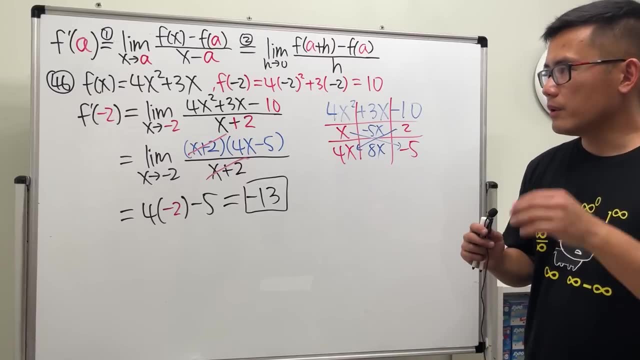 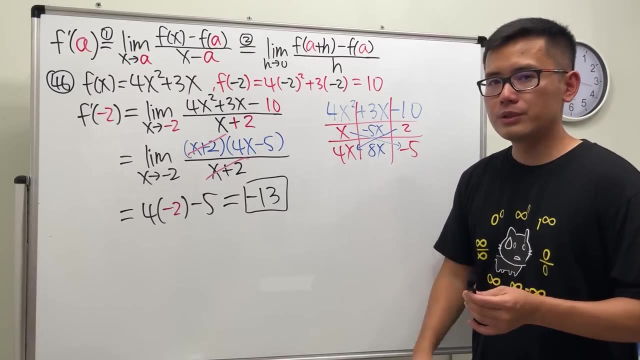 negative 8 minus 5 is negative 13. done, cool, but wow, that's a lot of work. i wonder if there's a way for me to know if we did this right or not. yes, of course we can do this question in like five seconds. check this out. 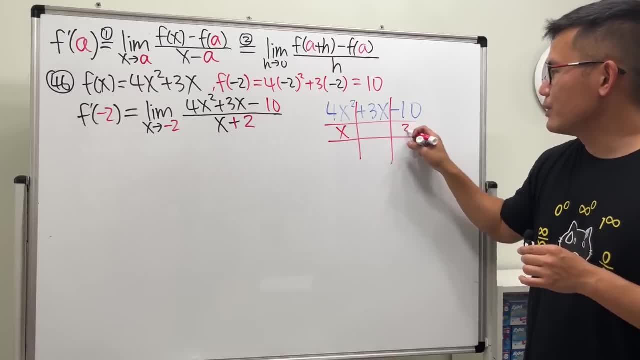 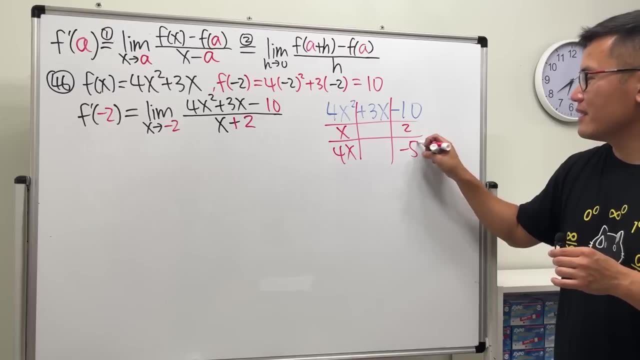 So you know the deal. We need to have x and 2 right here. 4x 2 times 4 will be negative, 10 is negative 5.. Why does this work? We need to get rid of that. Alright, So that's it, But check this out. 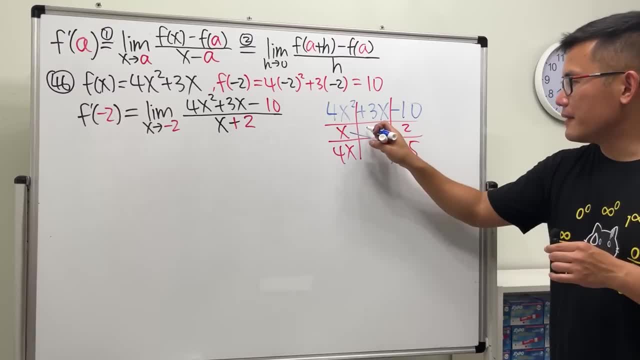 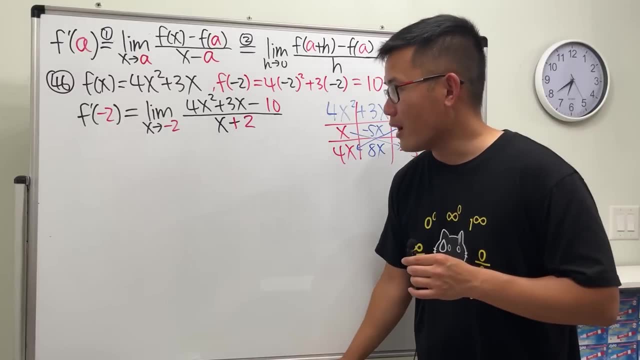 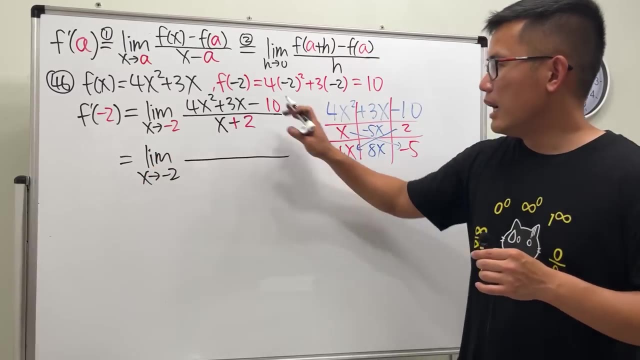 Check this out: x times negative 5 is negative 5x, and then 2 times 4x is 8x. Together, we do get the 3x that we want, Okay. So this is the limit as x approaching negative 2.. On the top, 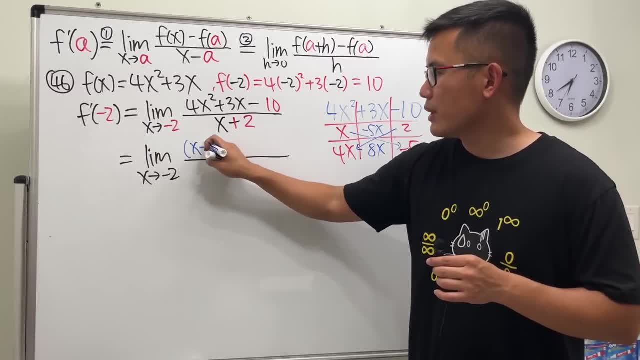 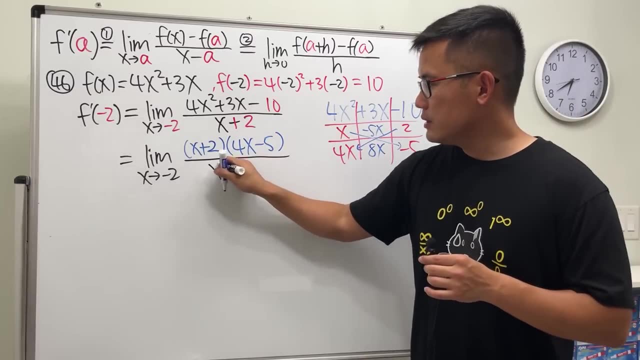 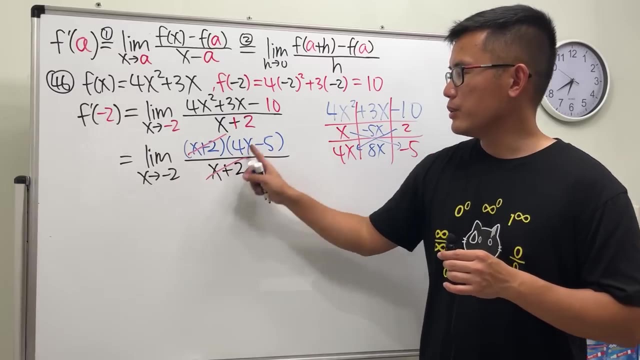 is just that, Namely x minus. So x plus 2 times 4x minus 5.. On the bottom is still x plus 2.. Overall, though, you see that this and that can cancel. Finally, put a negative 2 into here. 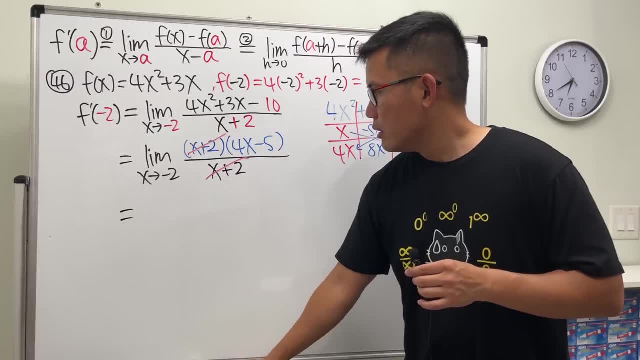 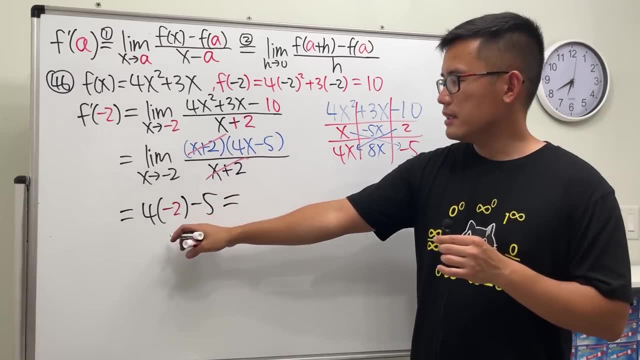 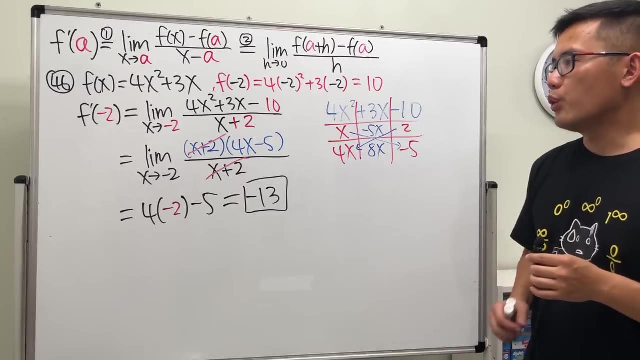 and we will get 4 times negative 2 and then minus 5.. Negative 8 minus 5 is negative 13. Done Cool, But wow, that's a lot of work. I wonder if there's a way for me to know if we. 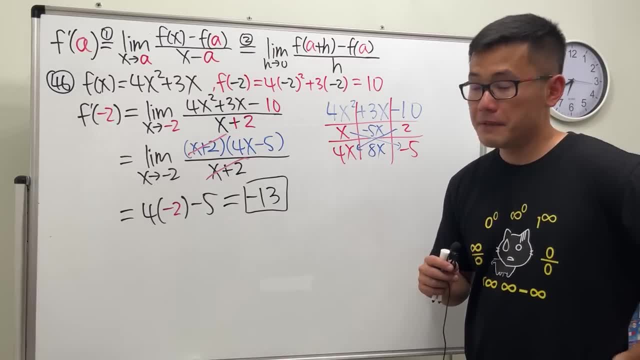 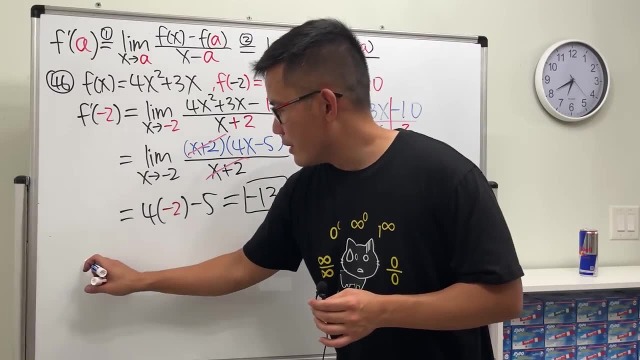 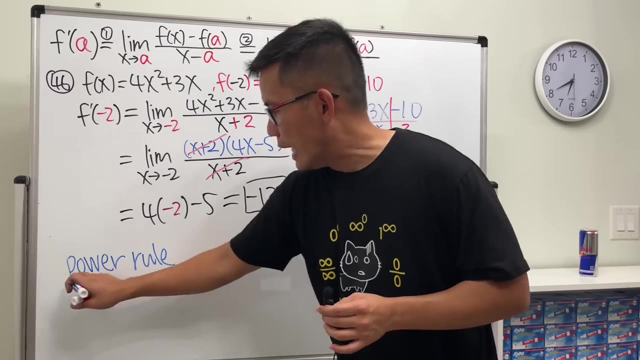 did this right or not? Yes, Of course, We can do this question in like 5 seconds. Check this out Right? This is the definition of derivative. This is the so-called power rule. I will have to mention this along the way, because 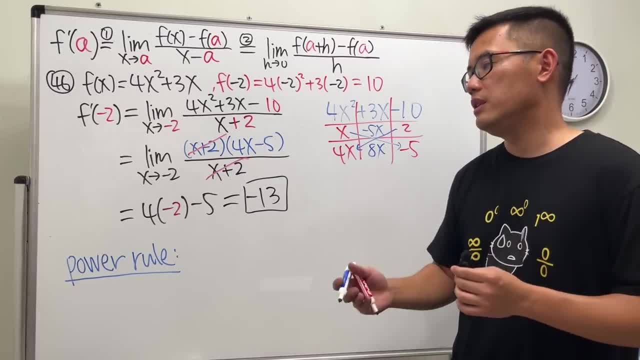 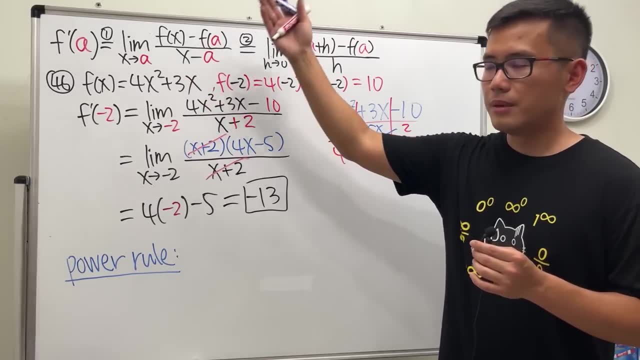 coming up. next we will be using the Lapito's rule, which we need the derivative. But if you are just learning derivative for the very first time, then please use the definition. Anyway, this is how it goes. Start with f of x. 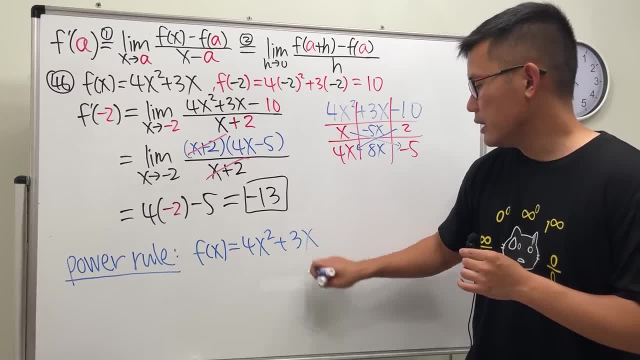 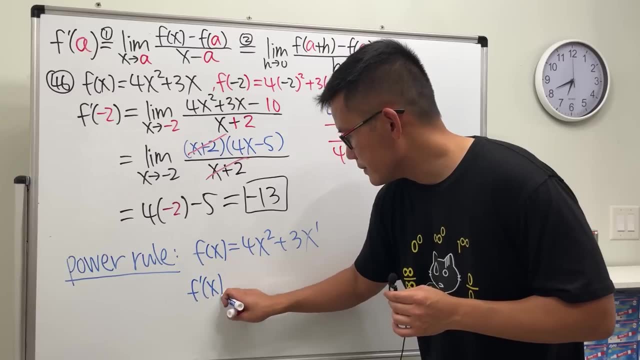 equals 4x squared plus 3x, And 3x is like the 3x to the first power. I will show you how it goes To get f prime of x whenever we have x to some power right here, not on the bottom. 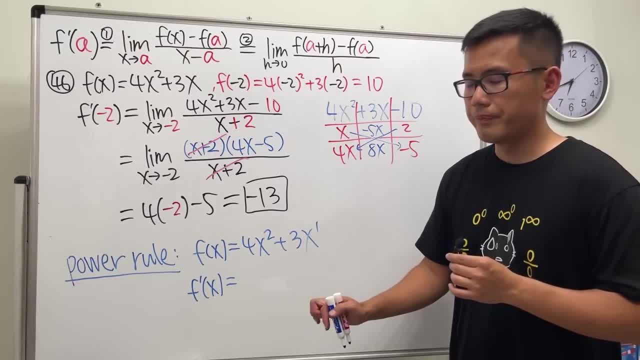 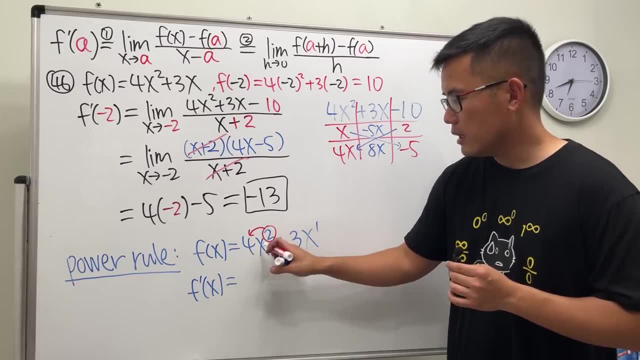 just right here. If you are multiplying by some number, that's good, That's cool. You can put the power to the front and multiply the 2 with that And then minus the power, Minus 1 to the power. So this right here will give us: 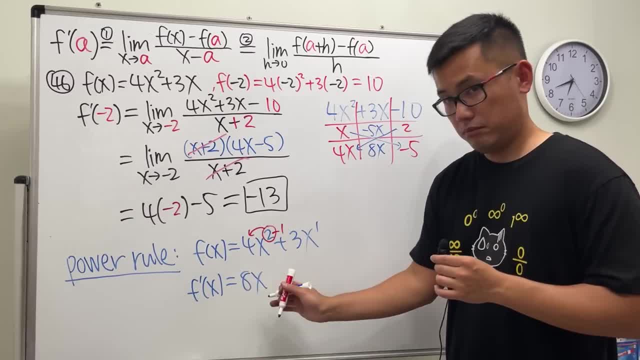 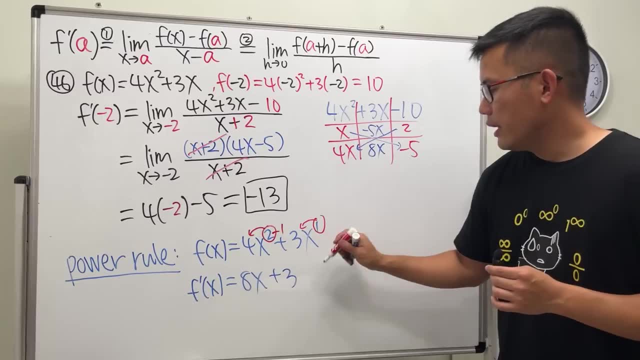 4 times 2 is 8.. x to the first power. Can we do the same thing for this one? Yes, Put the 1 to the front. 3 times 1 is 3.. And then don't forget to minus 1. 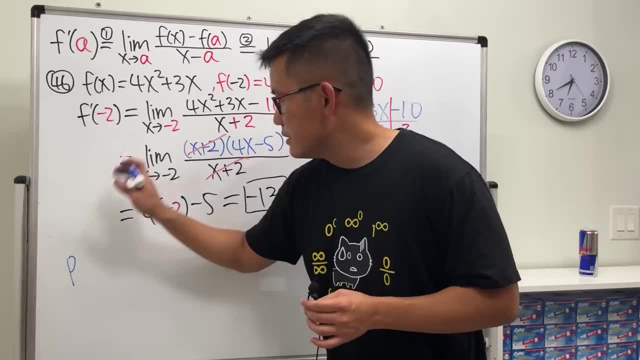 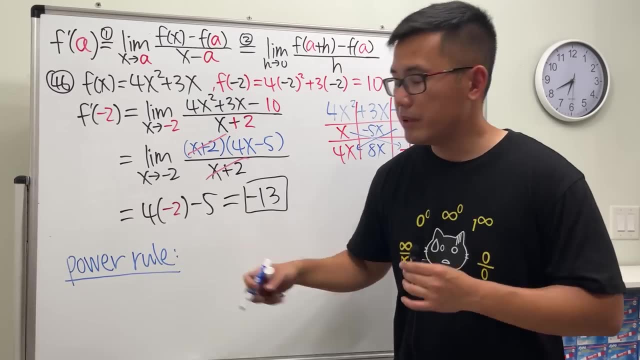 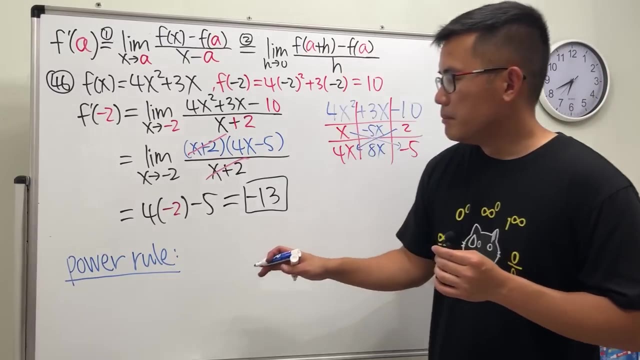 all right, this is the definition of derivative. this is the so-called power rule. i will have to mention this along the way because coming up next we will be using the lapidus rule, which we need the derivative. but if you are just learning derivative for the very first time, 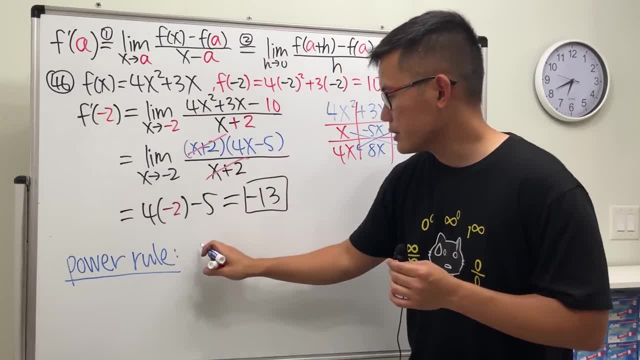 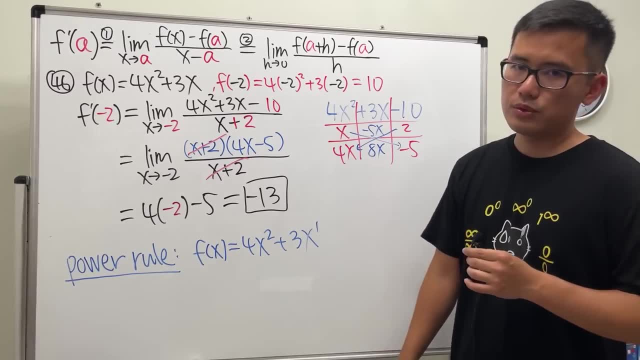 then please use the definition. anyway. this is how it goes. start with f of x equals 4x squared plus 3x, and 3x is like the 3x to the first power. i will show you how it goes to get f prime of x. 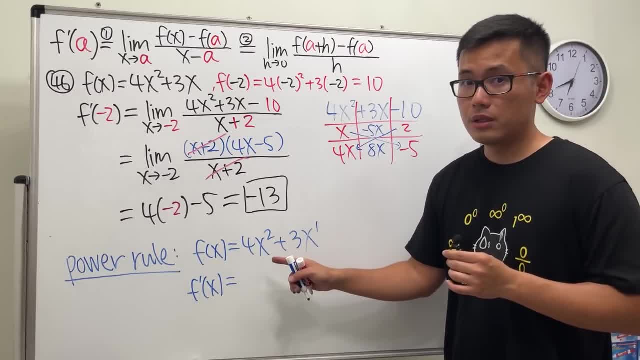 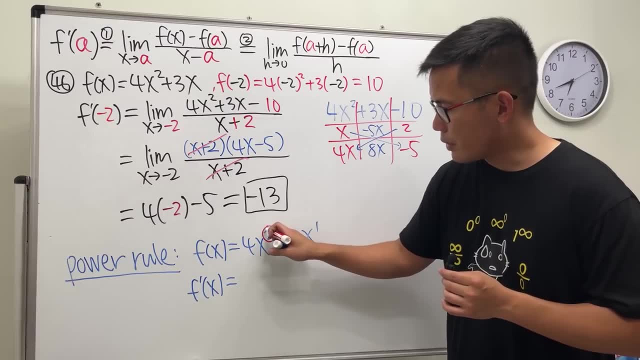 whenever we have x to some power right here, not on the bottom, just right here, huh. if you are multiplying by some number, that's good, that's cool. you can put the num, put the power to the front, and multiply with this, multiply the two with that and then minus the power. 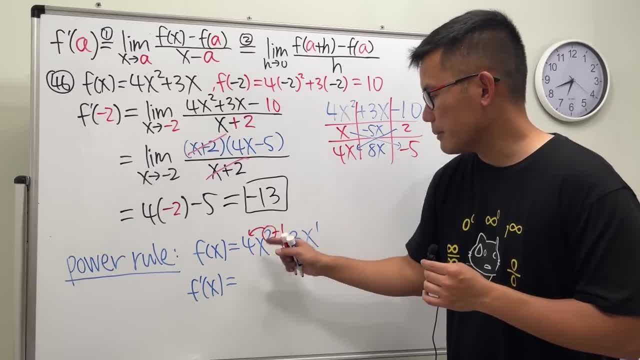 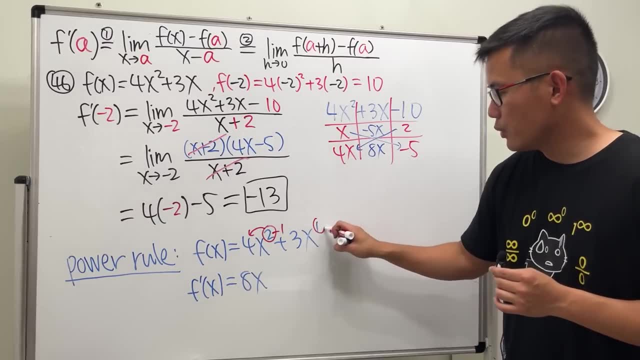 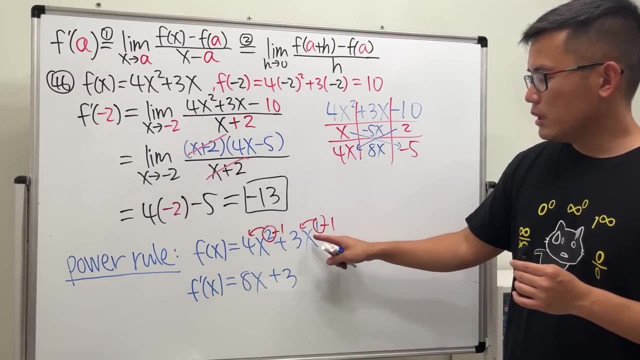 so my minus one to the power. so this right here will give us four times two eight x to the first power. can we do the same thing for this one? yes, put a one to the front. three times one is three. and then don't forget to minus one to the power. one minus one, zero. 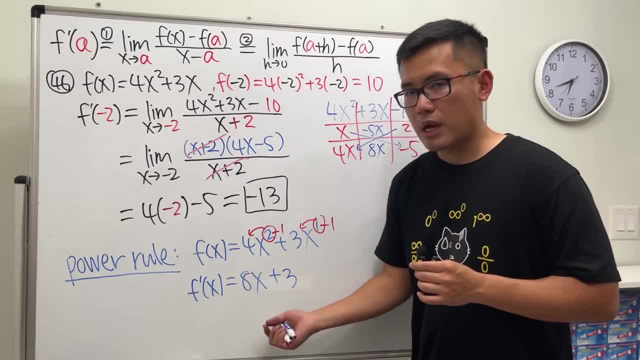 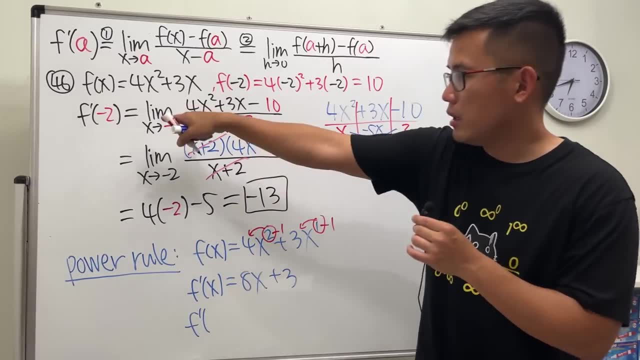 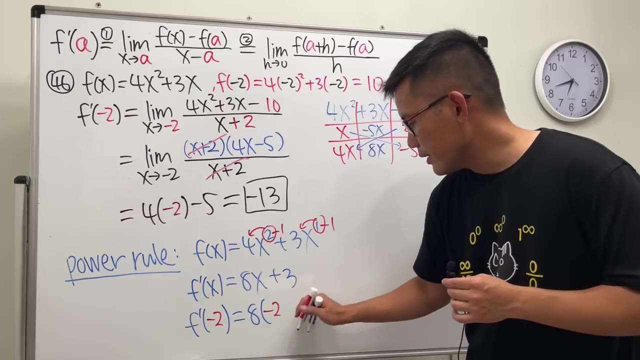 x to zero's power is one. so this is our f prime of x. it's so cool because now we can just plug in negative two that we wanted. so f prime of negative two is eight times negative two plus three. you bet it is negative thirteen done. 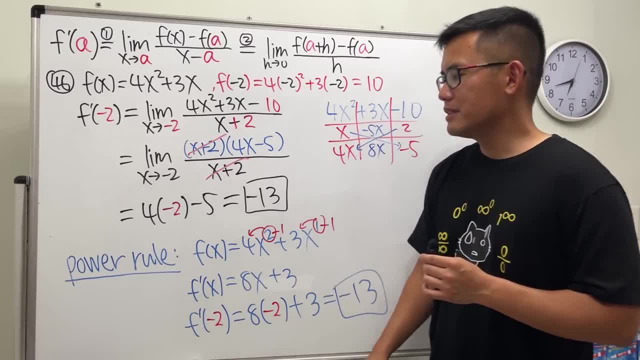 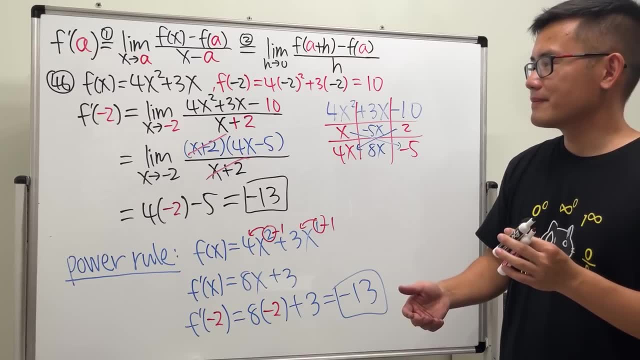 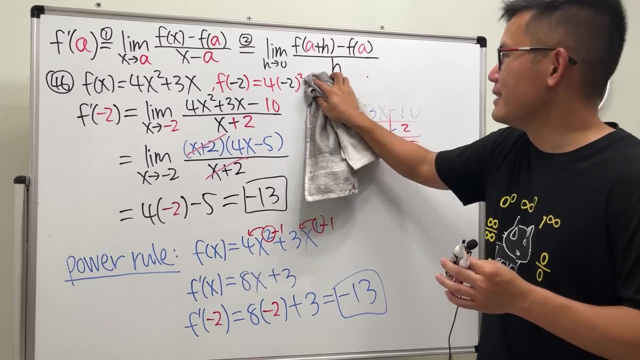 power rule. but don't be too happy about it, because knowing the power rule is not knowing all the calculus. this is a nice result. after the definition of the gravity, i'll say, all right, i want to make sure that i didn't. i'm gonna have to make sure that i am not. 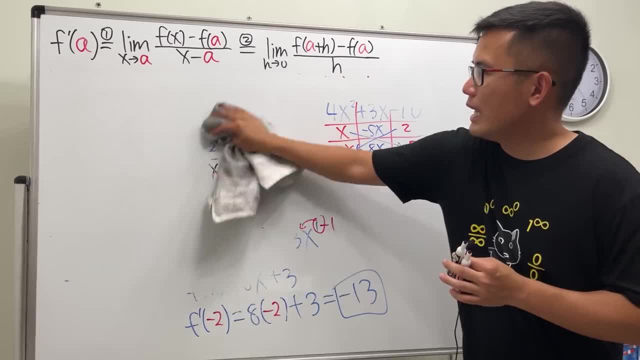 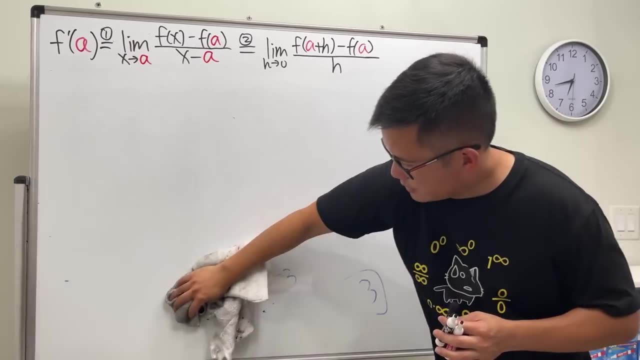 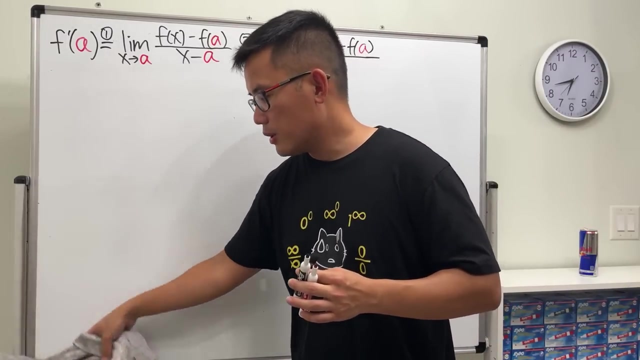 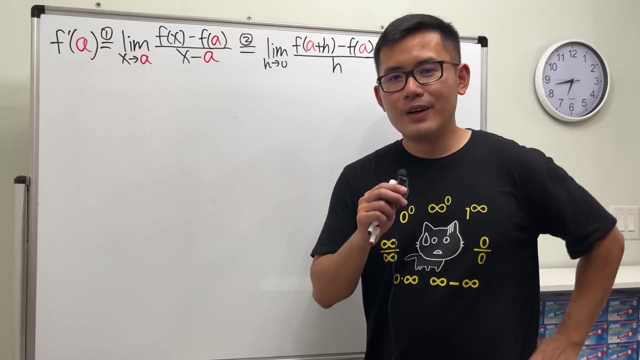 erasing the definitions because i would like to have them on the board until the end of the category and until this category. if you guys need help with derivatives, yes, you know it. we have the 100. we have had 100 derivative. took me a long time. 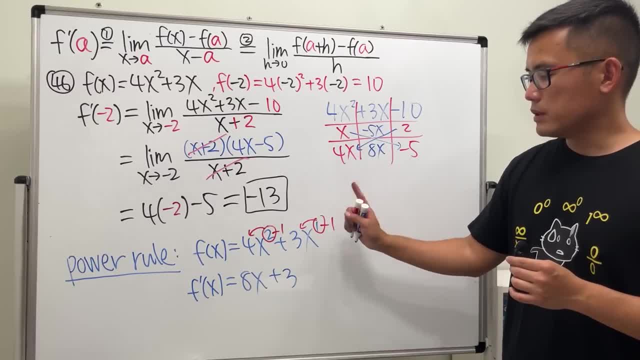 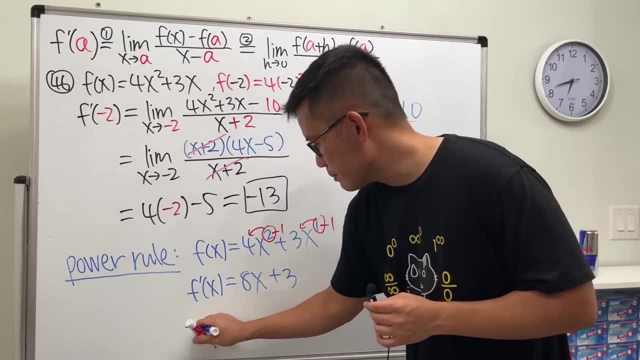 to the power, 1 minus 1 is 0.. x to 0's power is 1.. So this is our f prime of x. It's so cool Because now we can just plug in negative 2 that we wanted. 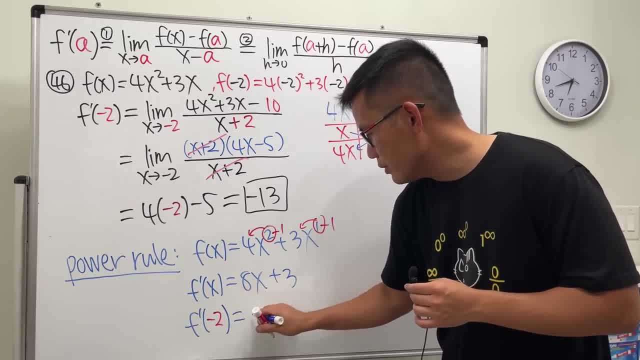 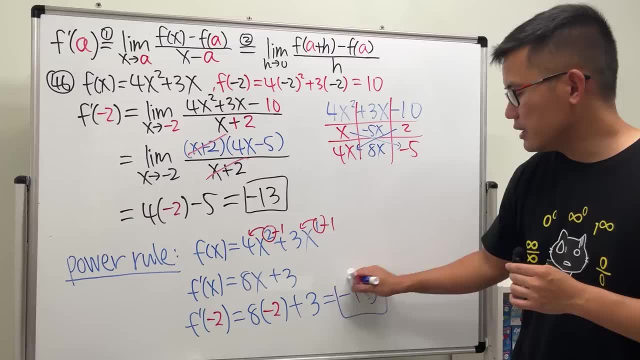 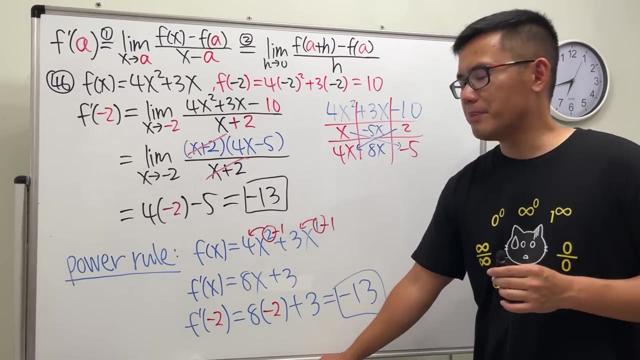 So f prime of negative 2 is 8 times negative 2 plus 3. You bet it is negative 13. Done Power rule, But don't be too happy about it, because knowing the power rule is not knowing all the calculus. 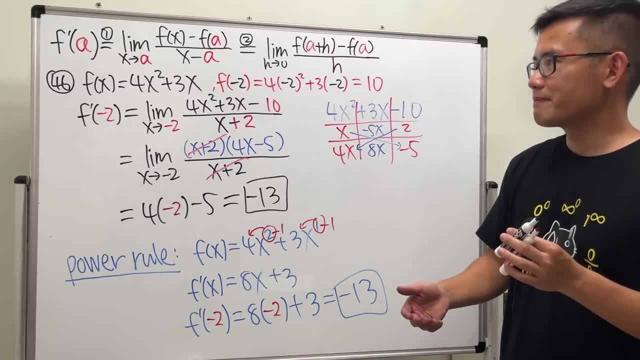 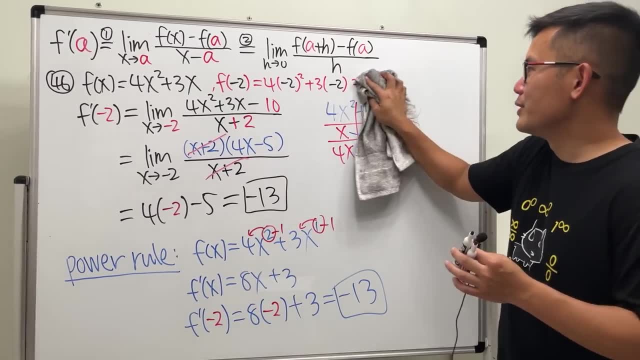 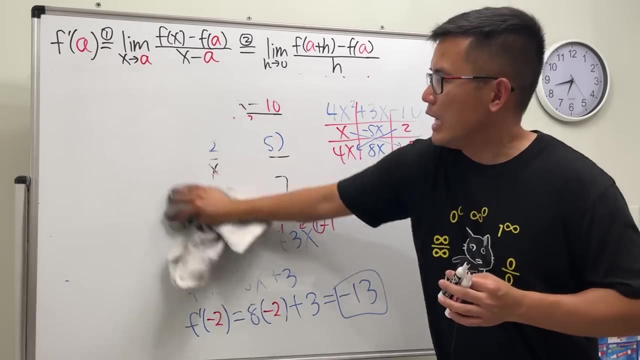 This is a nice result after the definition of the word for the outside. Alright, I want to make sure that I didn't. I have to make sure that I am not erasing the definitions because I would like to have them on the board until the end of the. 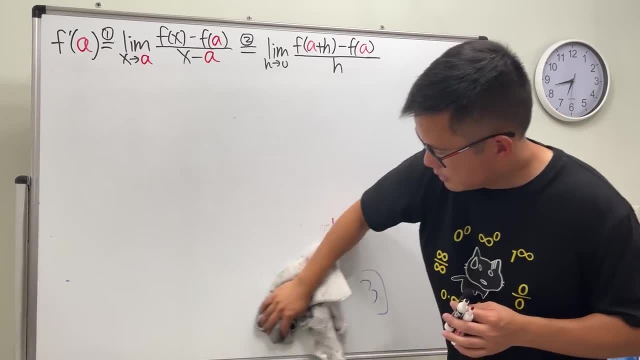 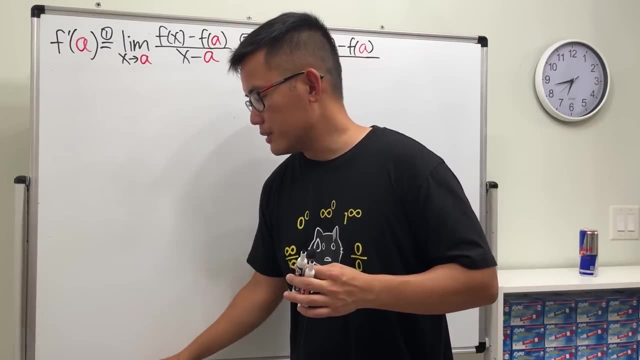 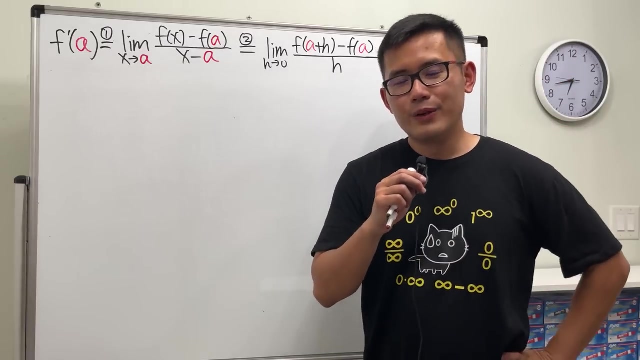 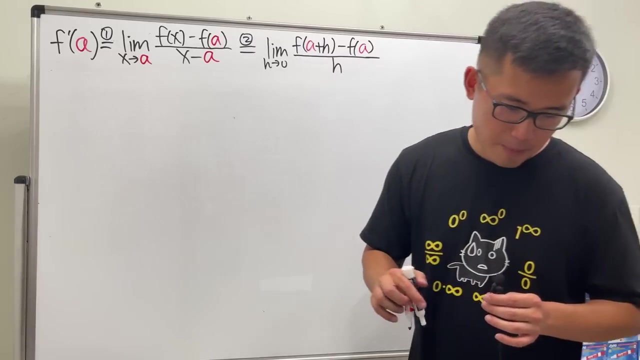 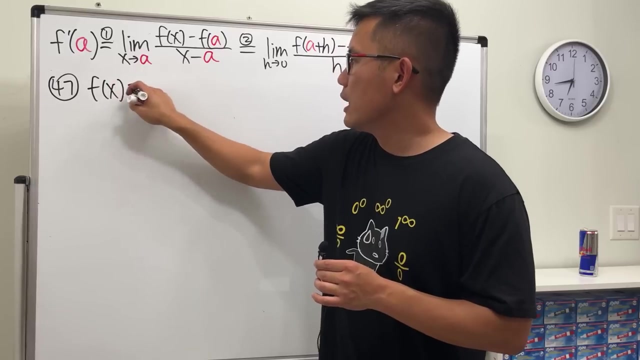 category. until this category. If you guys need help with derivatives, Yes, You know, We have the 100th derivative. Took me a long time to do that as well. Anyway, Number 47.. Okay, Function x over x plus 2.. We want. 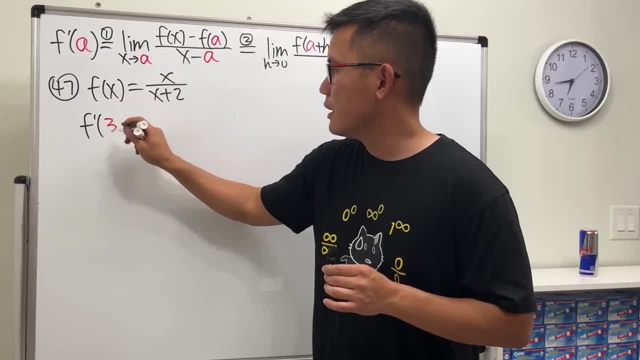 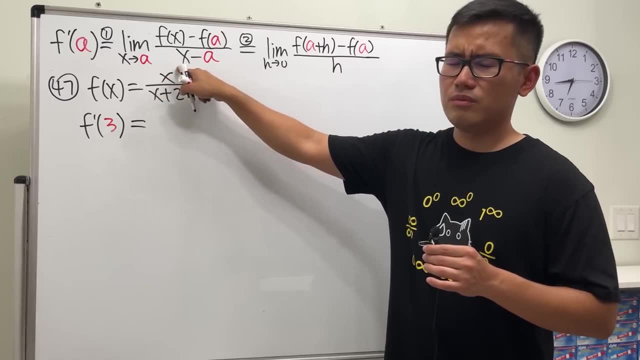 f, prime of 3.. Hey, Can we do the power rule? If we put a 1,, 1, bring the 2 of 1.. 1 minus 1 is 0.. x plus 0 is 1.. So we just get. 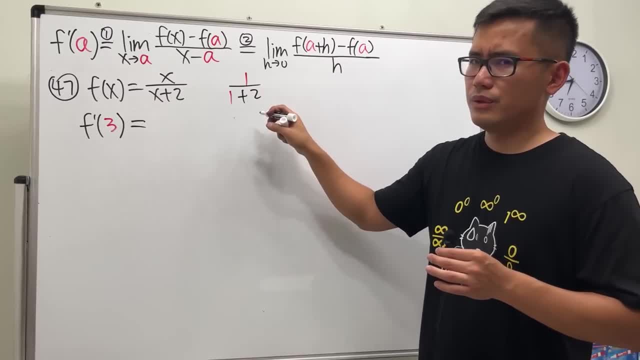 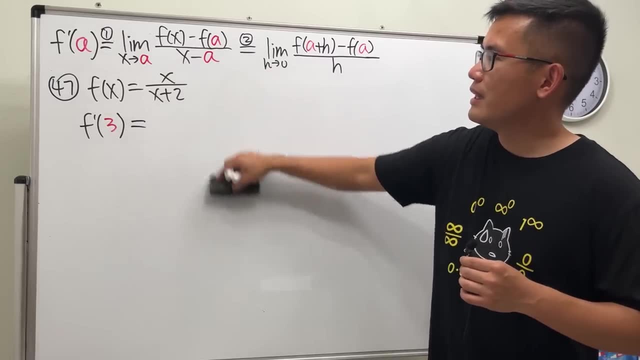 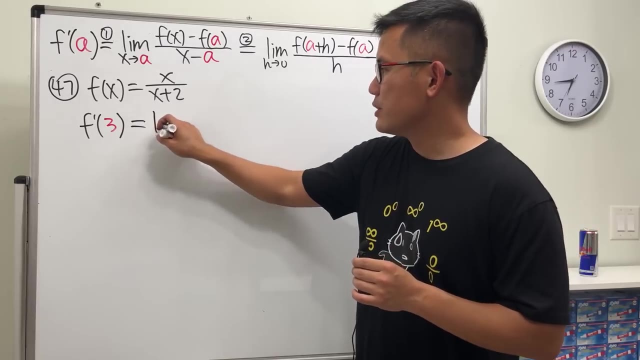 1 and then 1 plus 2.. The answer is just 1. third, No, No, Don't do that. That's why definition of derivative is the key Alright, Especially to take care of us when we are trying to do something. 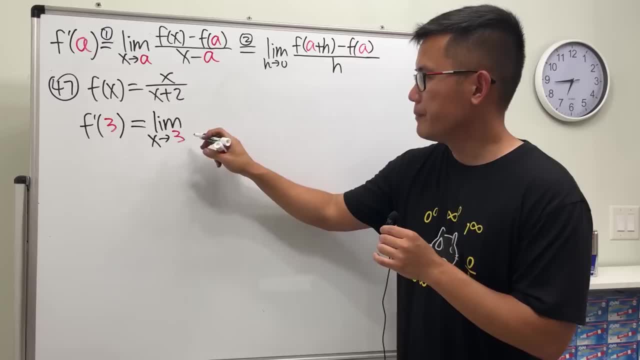 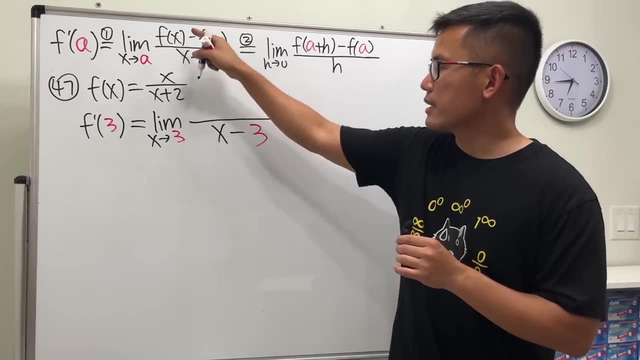 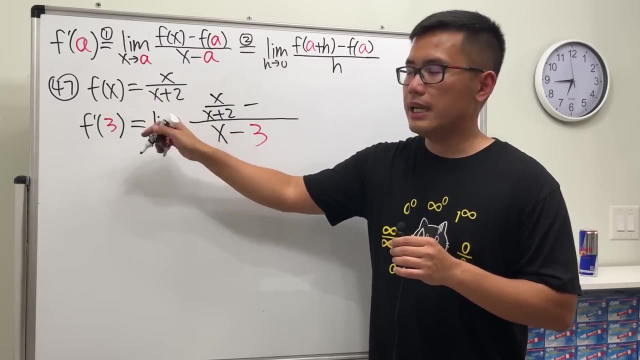 new The limit as x approaches 3.. We are following the first definition. We get x minus 3. And then on the top f of x is that So it's just x over x plus 2. And then minus, We have to put f of 3.. 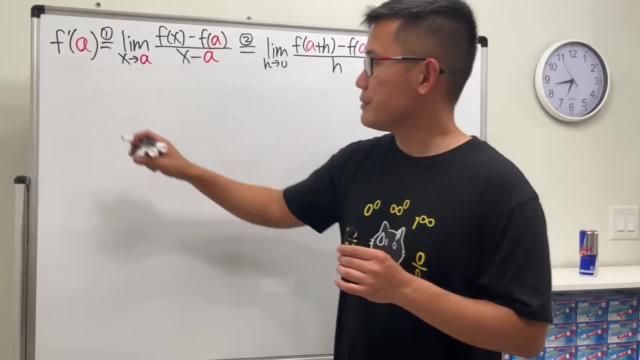 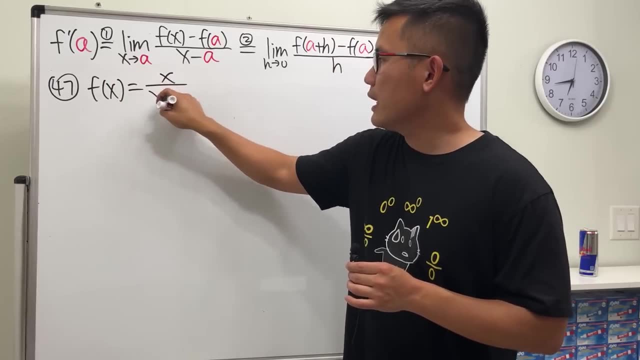 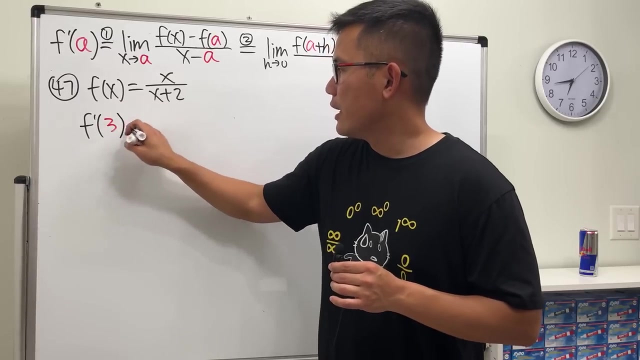 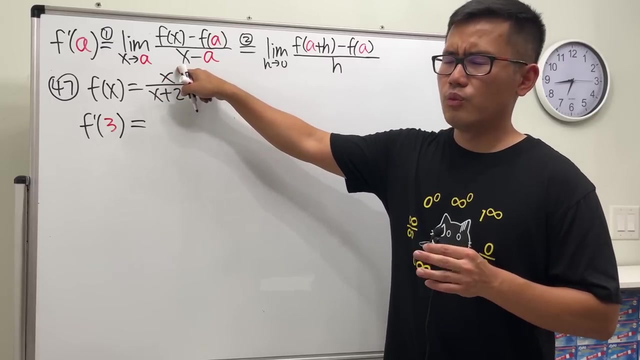 time to do that as well. anyway, number 47: okay, function x over x plus two. we want f prime of three. hey, can we do the power rule. if we put a one, one bring the two of one, one minus one, zero. x plus zero is one, so we just get one. 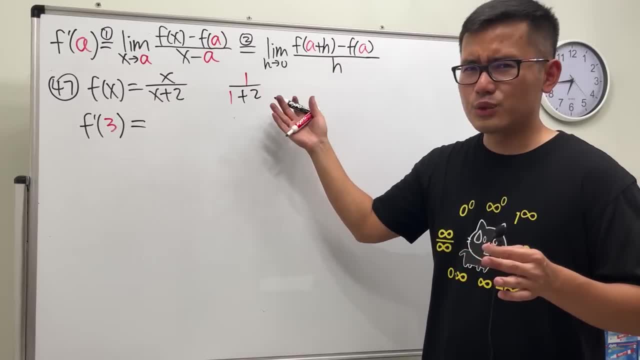 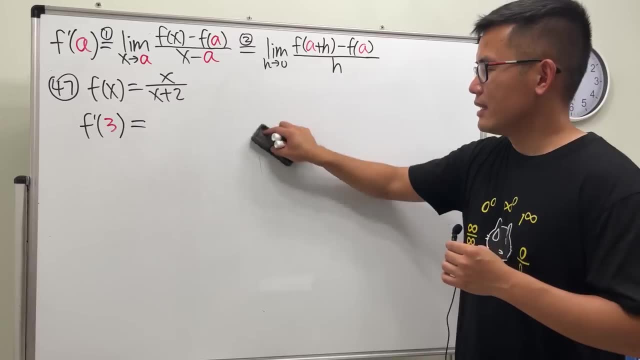 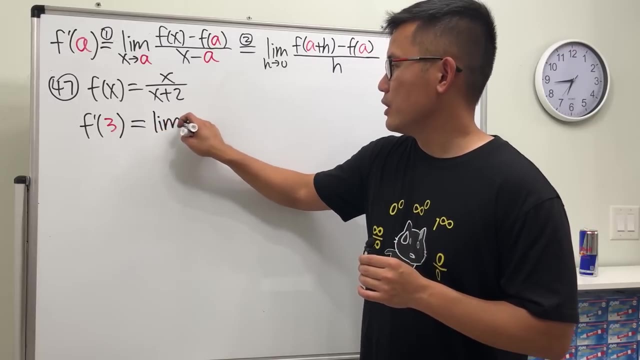 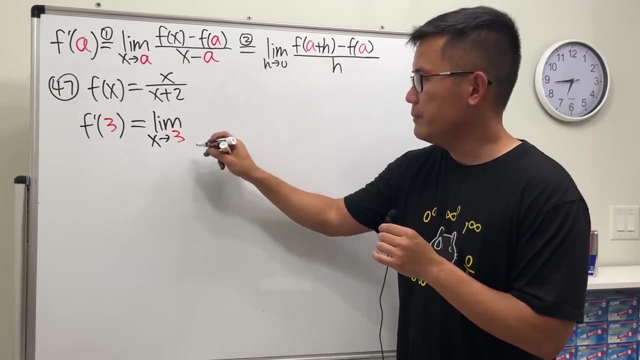 and then one plus three, two, the answer is just one third. no, no, no, no, no, don't do that. that's why definition of the rover is the key. all right, especially to take care of us when we're trying to do something new. the limit as x are portions three. right, we're following the first definition. 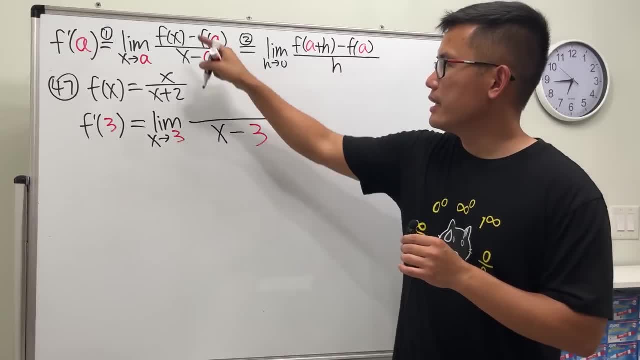 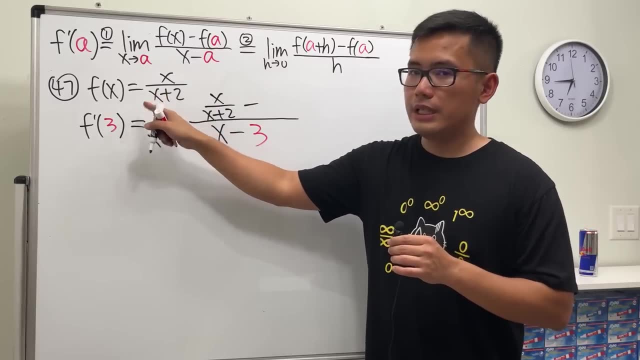 we get x minus three and then on the top, the first definition, we get x minus three. and then i'm going top: f of x is that so it's just x over x plus 2 and then minus. we have to put f of 3. yeah. 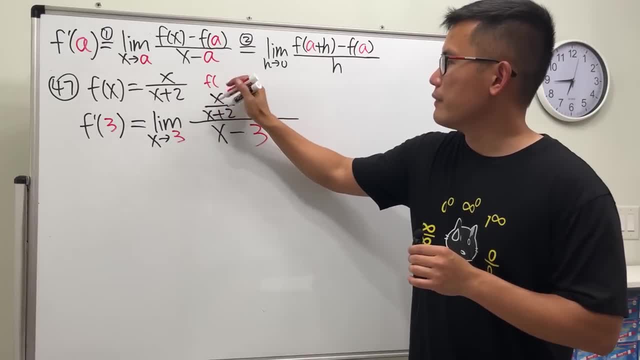 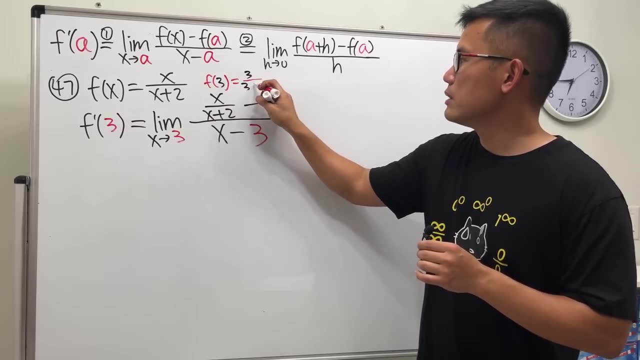 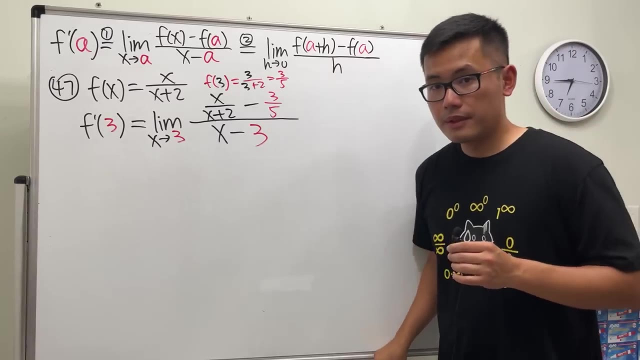 so i'll just indicate that right here. f of 3 is just 3 over 3 plus 2, so it's just 3 over 5, so it's minus 3 over 5.. okay, as we can see, we have a complex fraction. 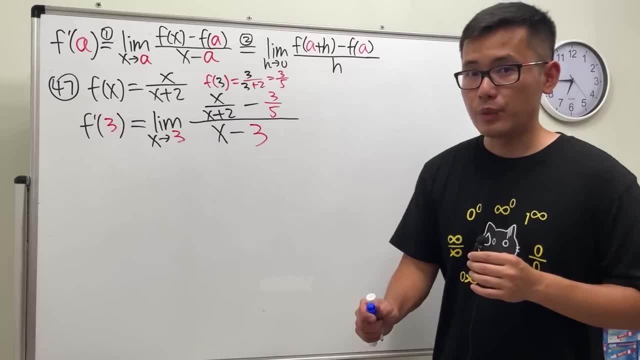 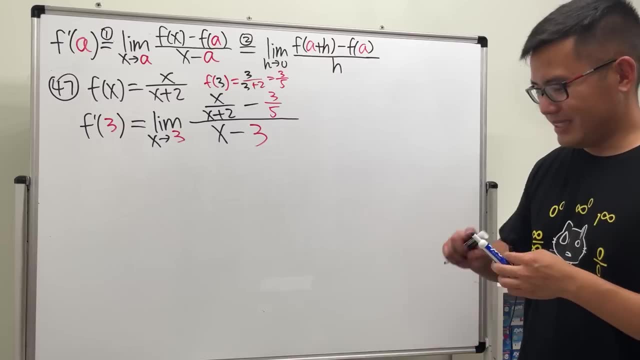 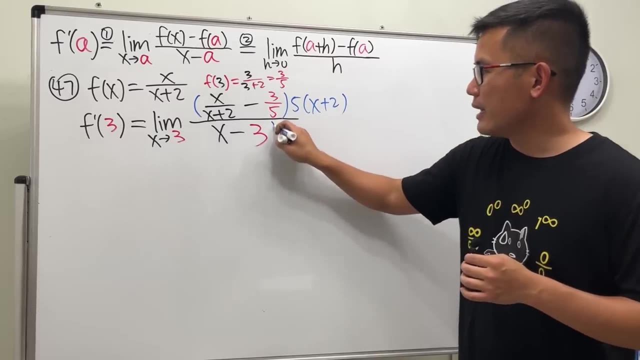 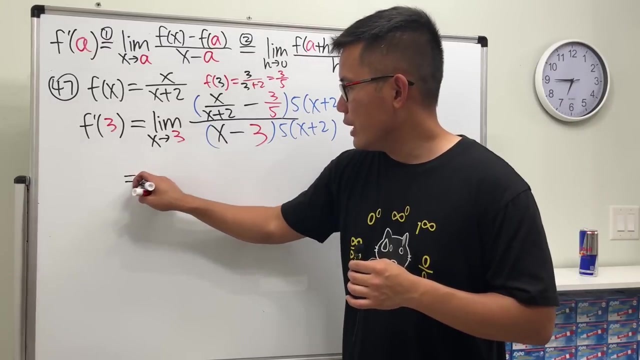 situation. therefore, we are going to do the things that we did right. that's why we talk about the algebraic ways to to the limits. i'm going to multiply the top and bottom by this and that, so it's 5 times x plus 2, and likewise here, 5 times x plus 2.. all right, here we are going to get a. 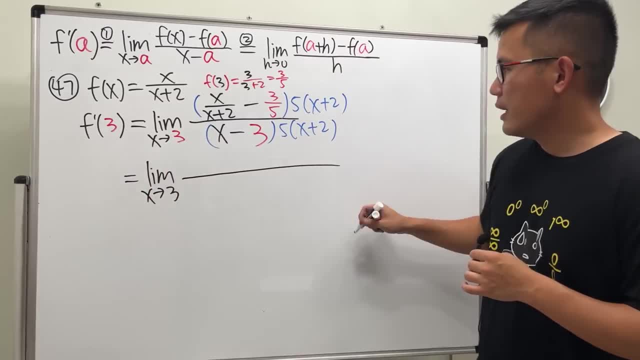 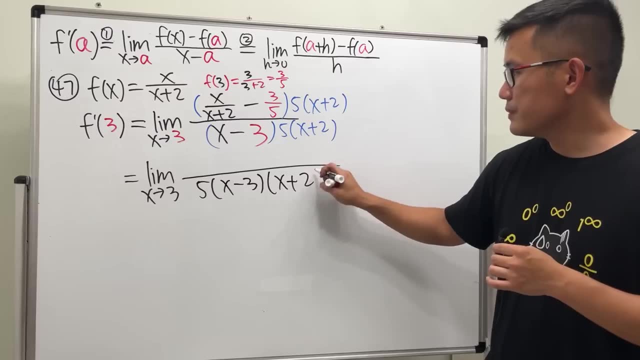 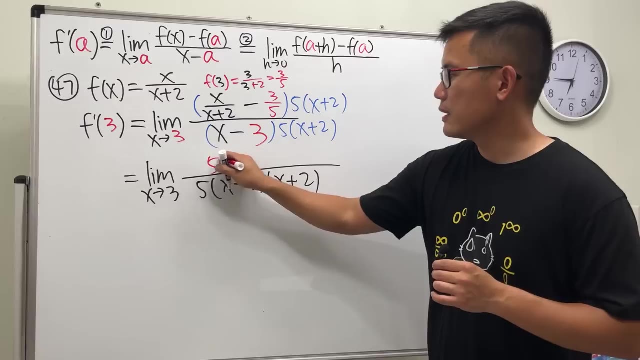 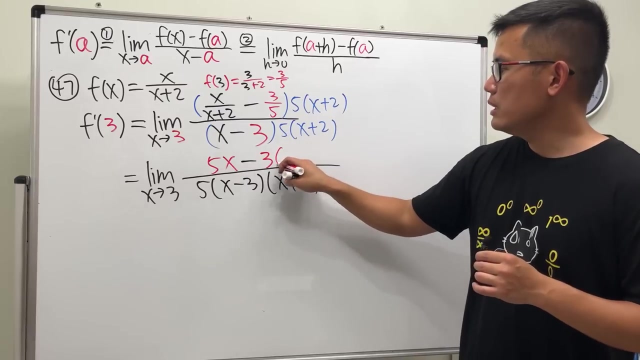 limit as x approaches 3.. let me just keep this how they are. so 5 and then x minus 3, x plus 2.. now let's multiply at the top, this times that x plus 2 cancel, so we have 5x minus 5 and 5 cancel, but we have this 3 and also the x plus 2, am i right? let me just double check. 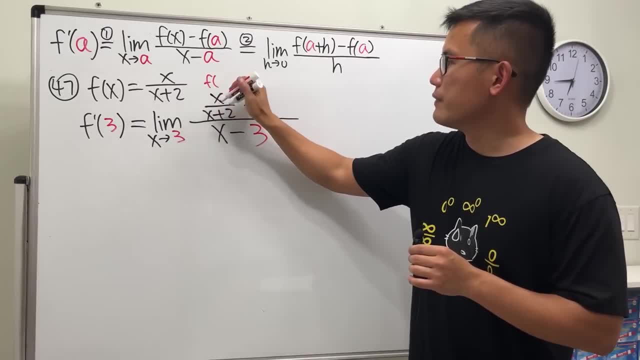 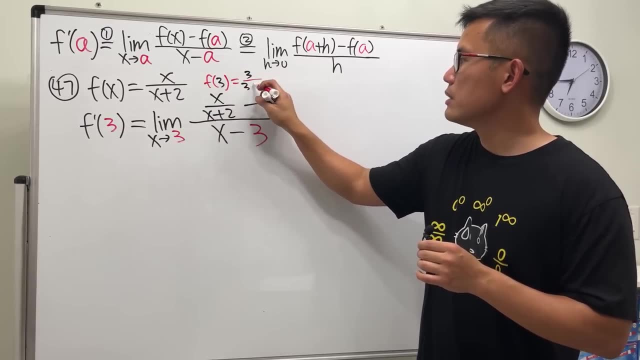 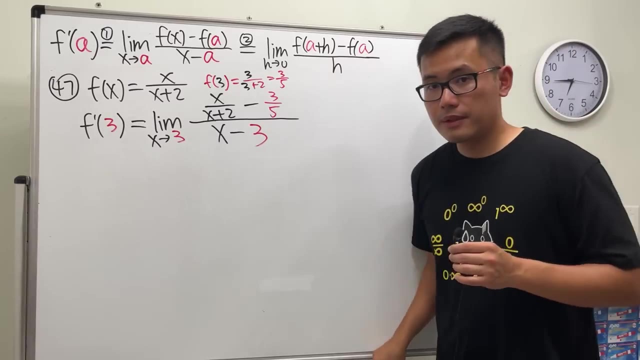 So I will just indicate that right here: f of 3 is just 3 over 3 plus 2. So it's just 3 over 5.. So it's minus 3 over 5.. Okay, As we can see, 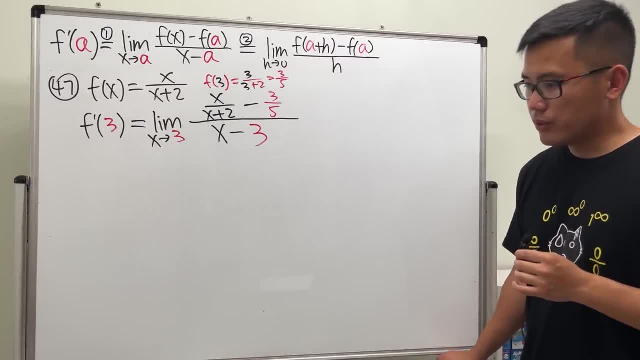 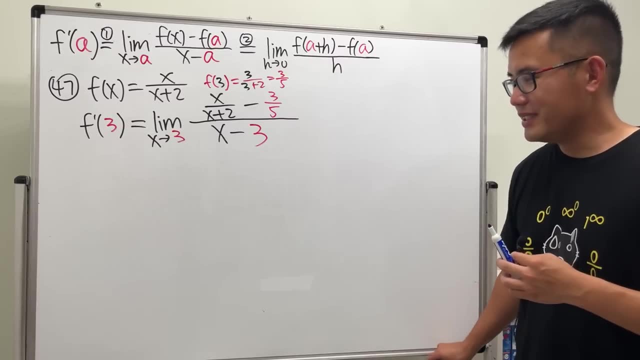 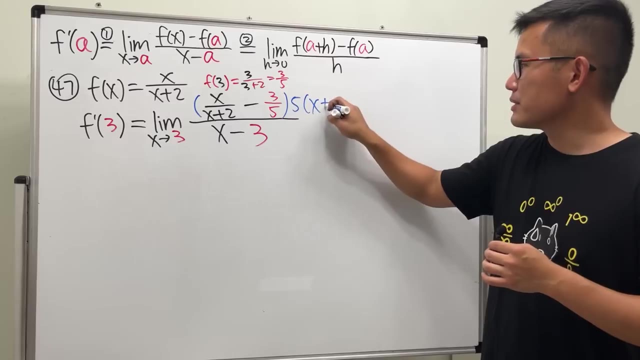 we have a complex fraction situation. Therefore, we are going to do the things that we did Right. That's why we talk about the algebraic ways to the limits. I'm going to multiply the top and bottom by this and that, So it's 5 times x plus 2.. 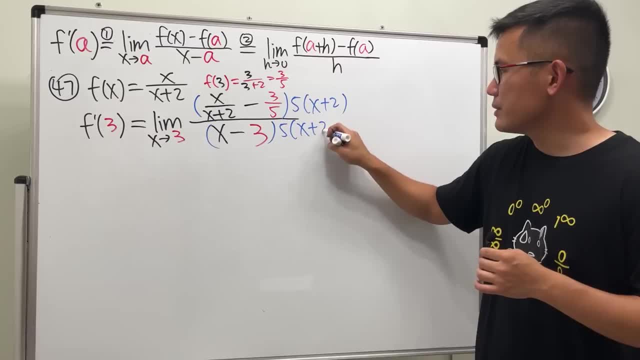 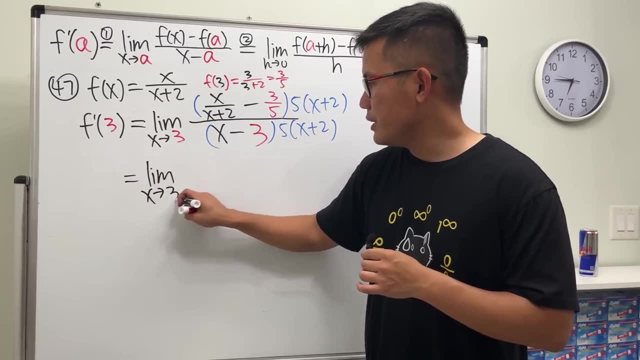 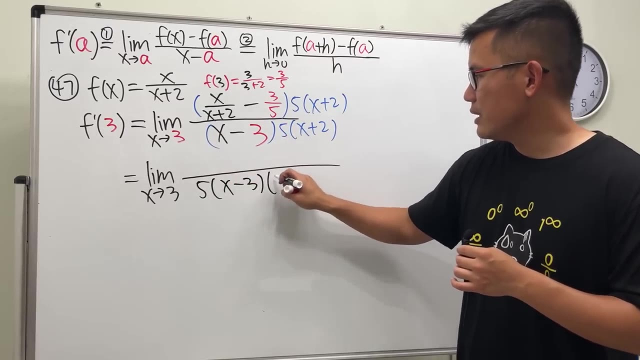 And likewise here, 5 times x plus 2.. Alright, Here we are going to get a limit As x approaches 3.. Let me just keep this how they are. So 5 and then x minus 3.. x plus 2.. 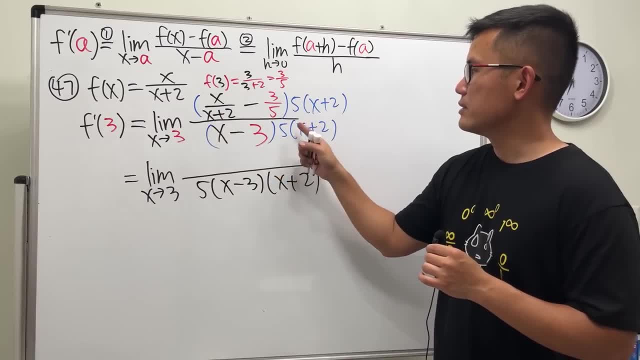 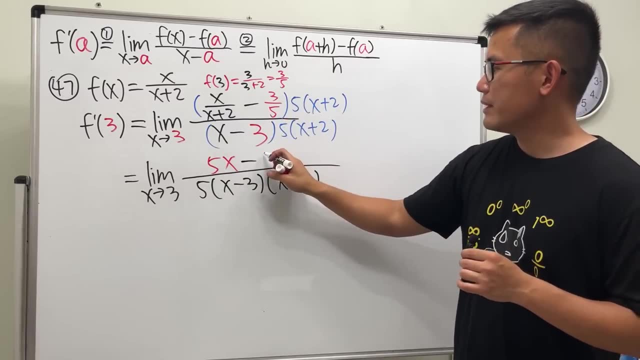 Now let's multiply the top. This times that x plus 2 cancel, So we have 5x Minus 5 and 5 cancel, But we have this 3. And also the x plus 2. Am I right? 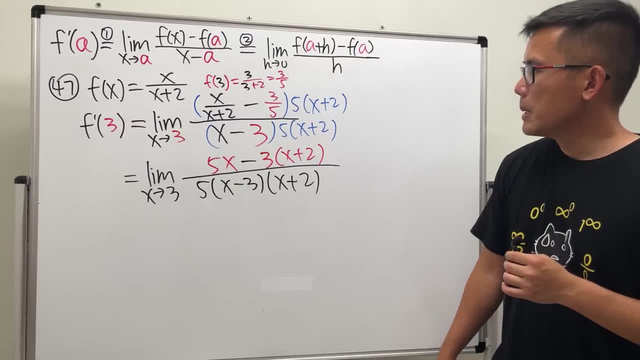 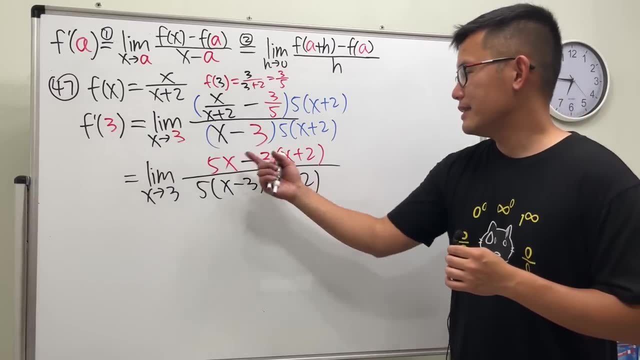 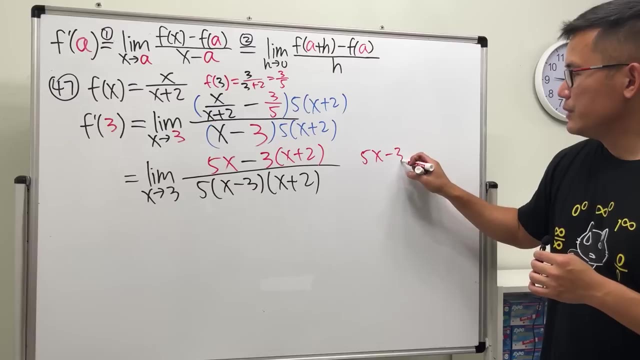 Let me just double check. Okay Cool, I didn't leave space on the top, So I'm just going to do it on the side. You see this is just 5x minus 3x and then minus 6.. So it's just 2x. 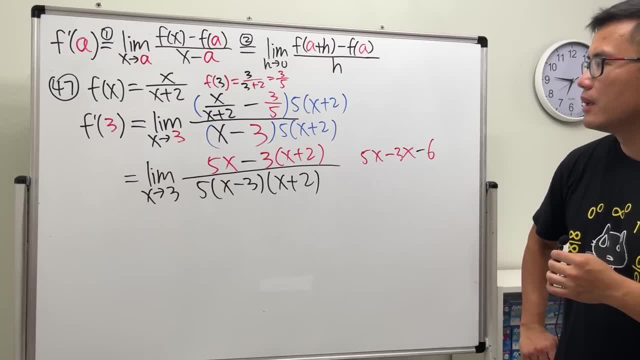 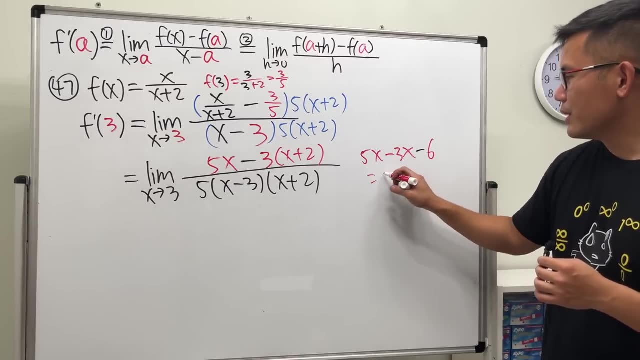 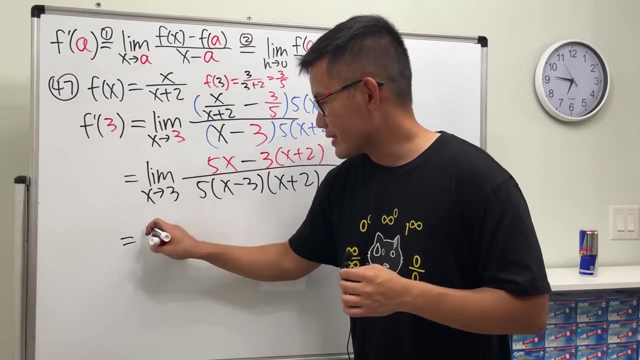 Hold on. Oh no, no, 2x minus 6.. So this right here is 2x minus 6. And then we can factor out the 2. So it's 2 times x minus 3.. So the top part. 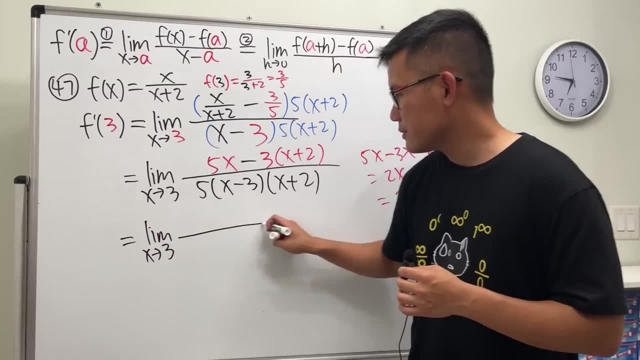 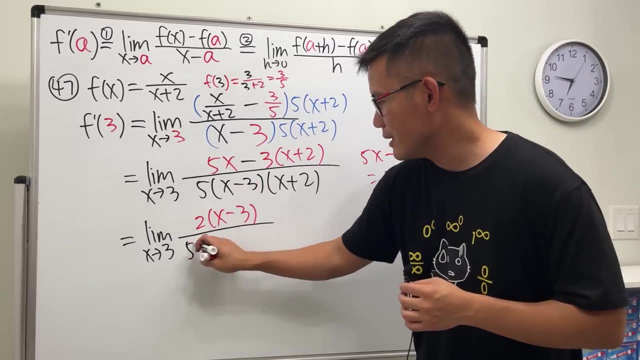 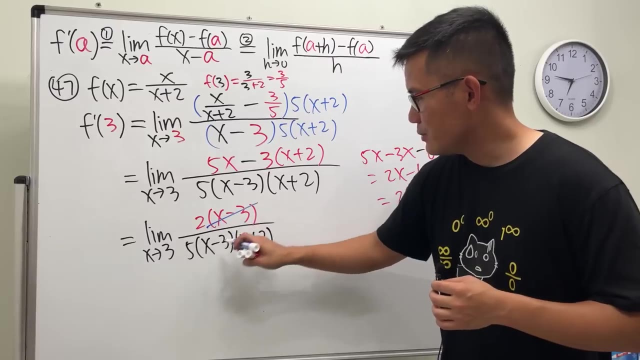 is that? So let me just rewrite this. So we get 2 times x minus 3.. And you see we can cancel things out on the bottom. So 5 times x minus 3.. x plus 2.. Very nice, Cancel. 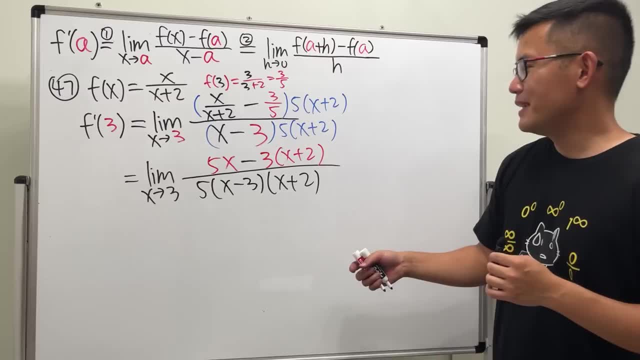 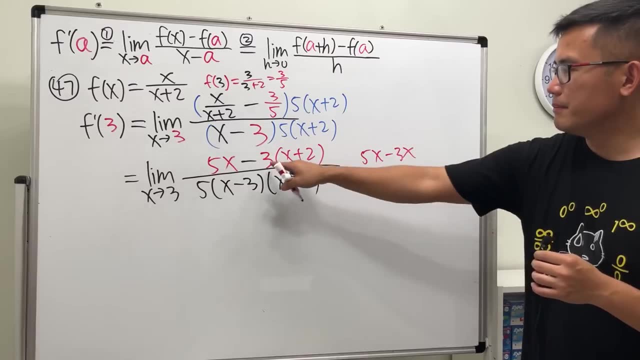 okay, cool, now i had. i didn't leave space on the top, so i'm just going to kind of do it on the side. so you see, this is just 5x minus 3x and then minus 6. yeah, so just 2x, hold on. 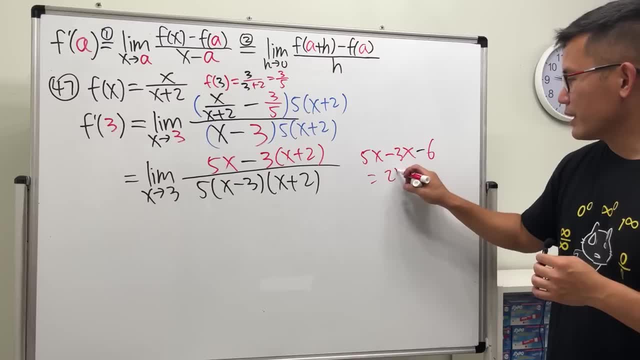 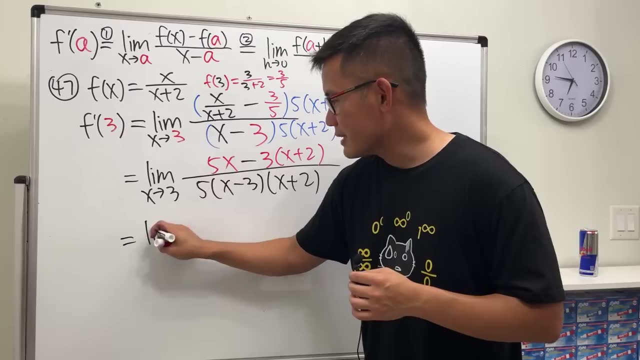 oh no, no, 2x minus 6.. so this right here is 2x minus 6, and then we can factor out the 2, so it's 2 times x minus 3.. okay, so the top on. so the top part is that. so let me just rewrite: 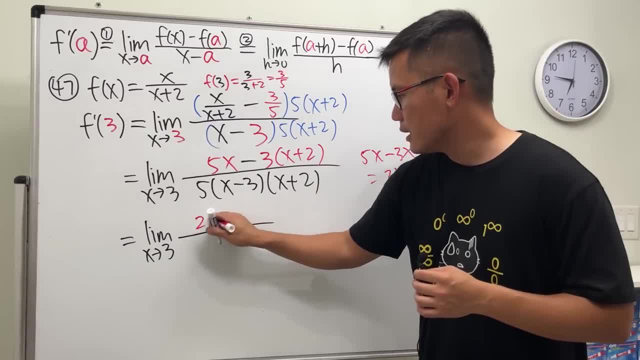 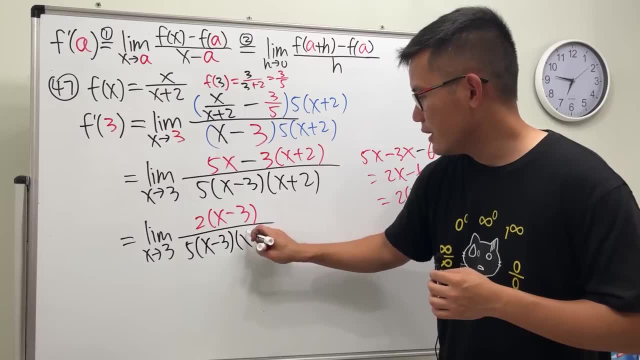 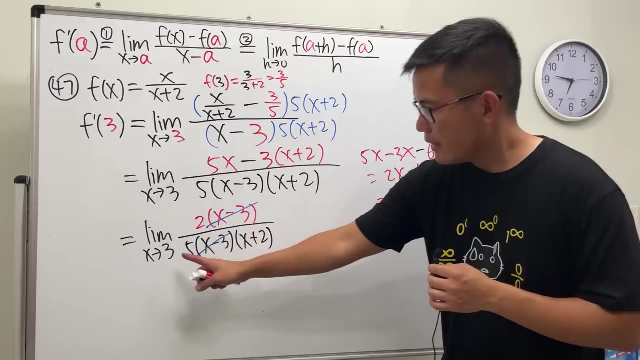 this. so we get 2 times x minus 3 and you see we can cancel things out on the bottom. so 5 times x minus 3 x plus 2. very nice, huh x minus 3, cancel. now put a 3 into here. so we are going to get. 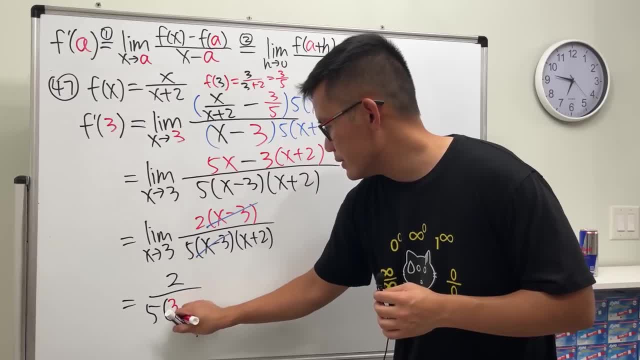 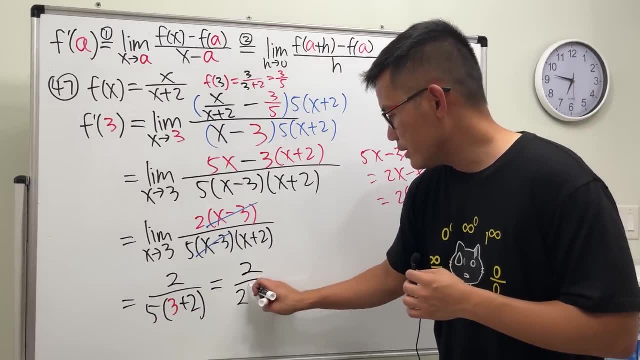 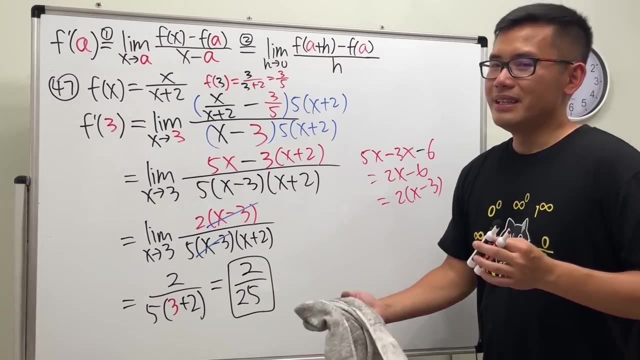 2 over 5 times 3 plus 2- that's 5 times 5, is 25. so altogether we get 2 over 25 done. it was not like power rule. yeah, you have to use the so-called quotient rule, but we're not going to get into that in this video. we have the 100. 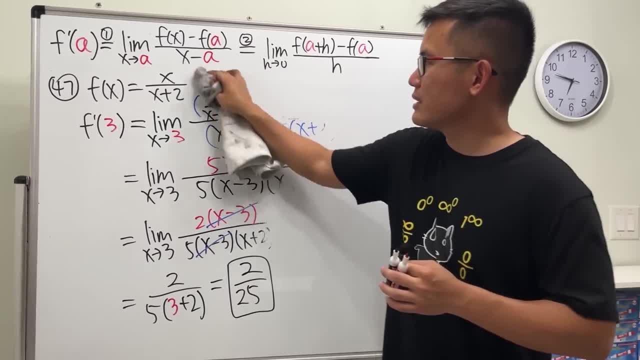 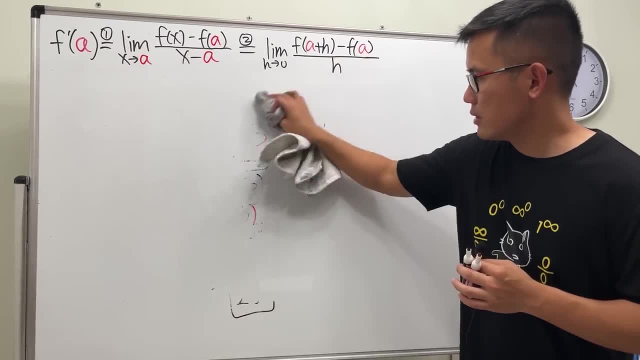 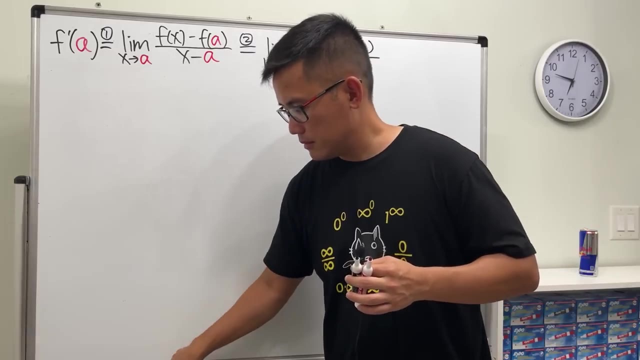 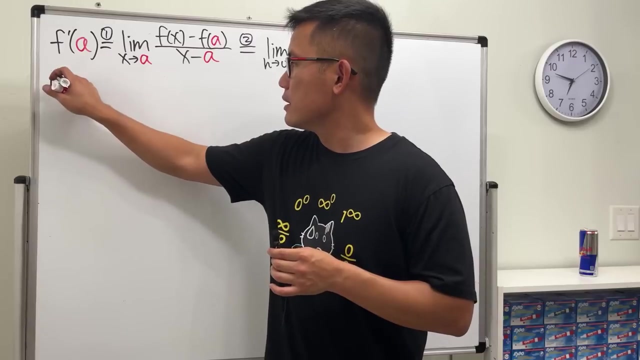 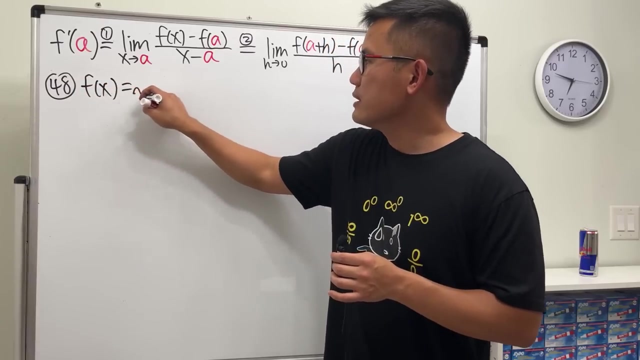 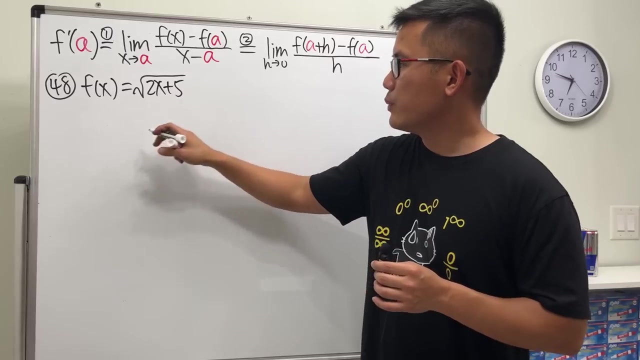 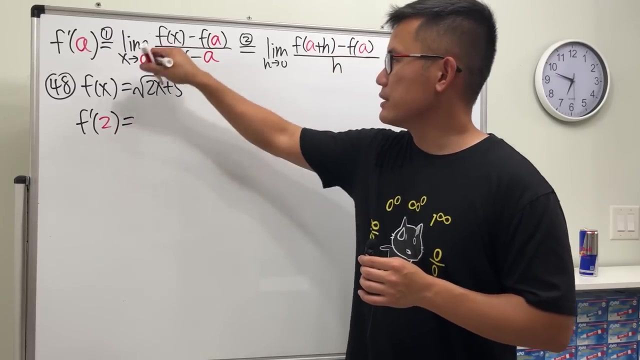 we have the 100 derivative for that already, so go ahead and check that out. so all right, number 48 let's talk about. let's take a look at this square root function: f of x equals square root of 2x plus 5.. and then we want f prime of 2 and let's just use the first definition. 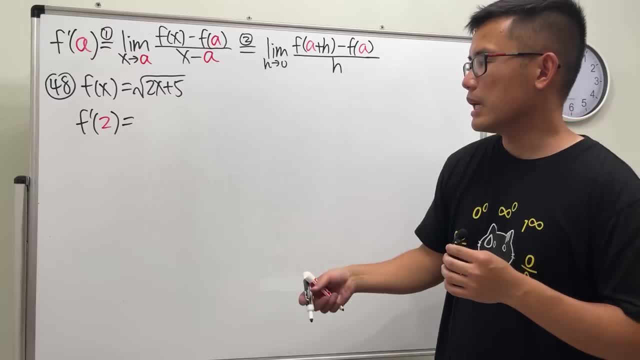 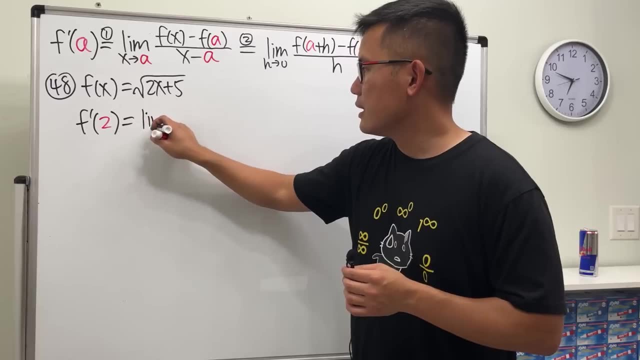 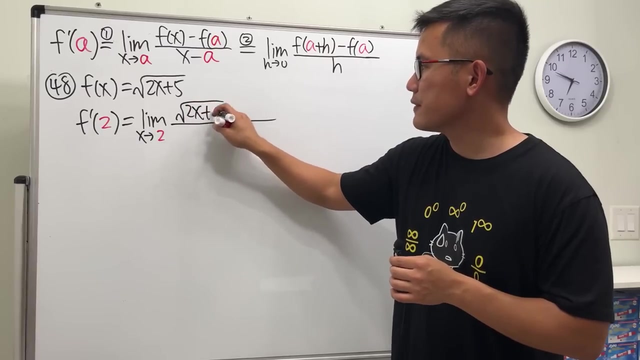 i think it's more straightforward, more direct this way, yeah, but this one also works. don't worry, we will have a chance to practice this data on, you'll see. anyway, this is the limit as x approaching 2. and then here we have our function square root of 2x plus 5.. and then here we have our function square root of 2x plus 5.. 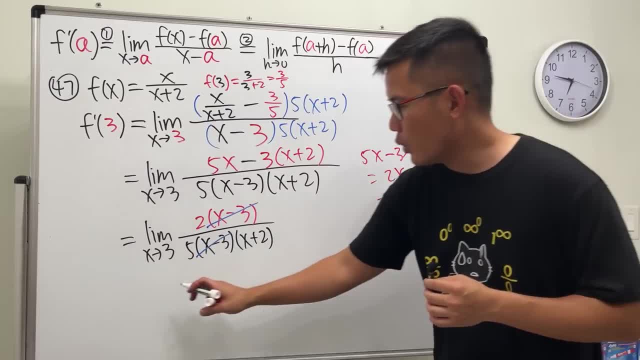 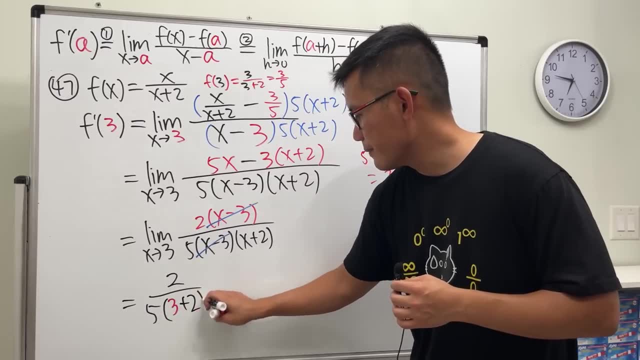 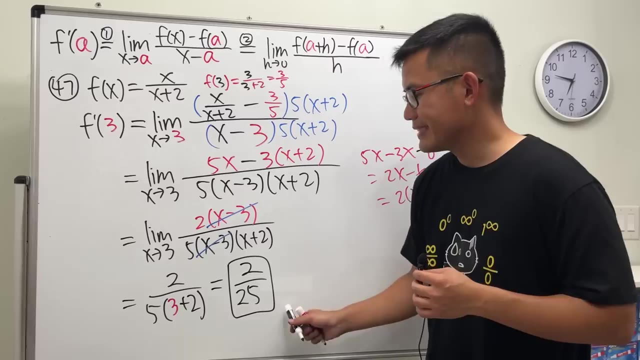 Now put the 3 into here, So we are going to get 2 over 5 times 3 plus 2. That's 5 times 5. It's 25.. So altogether we get 2 over 25.. Done. 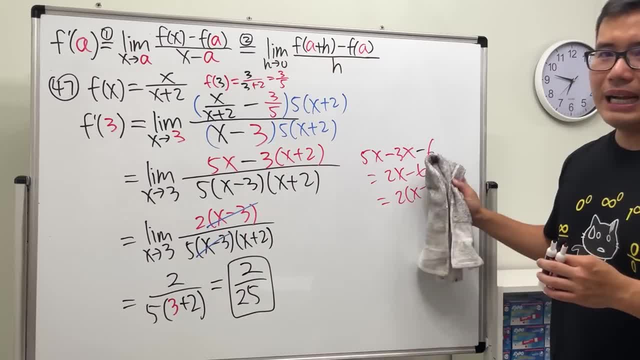 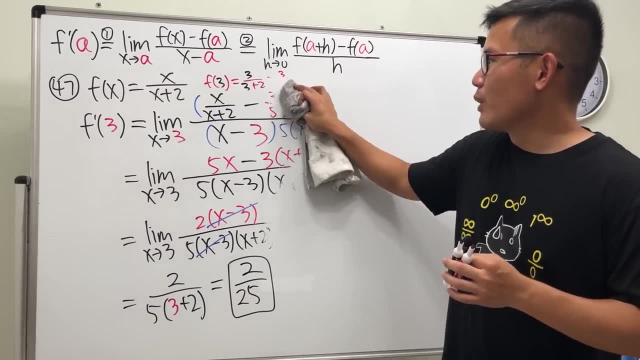 It was not like power rule. Yeah, you have to use the so called quotient rule, But we are not going to get into that in this video. We have the 100.. We have the 100 derivative for that already, So go ahead and check that out. 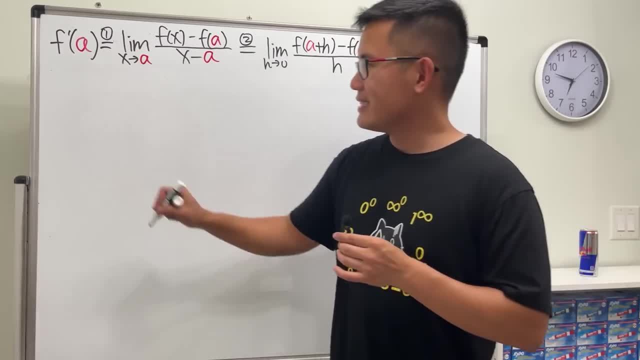 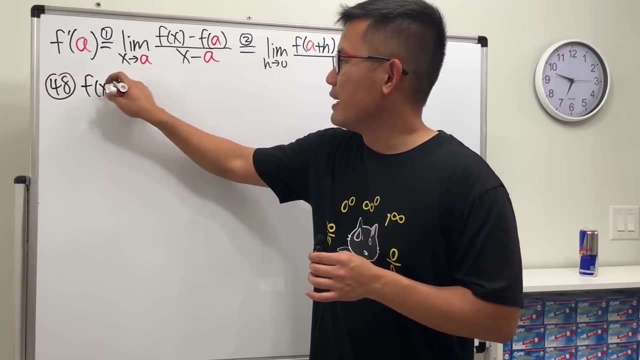 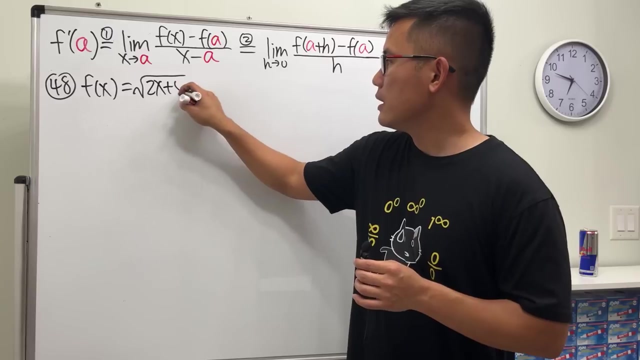 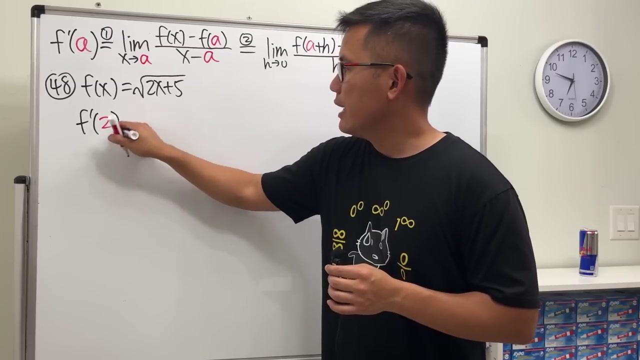 Alright, Number 48.. Let's talk about, Let's take a look at, the square root function. f of x equals square root of 2x plus 5.. And then we want f prime of 2.. And let's just use the first definition. 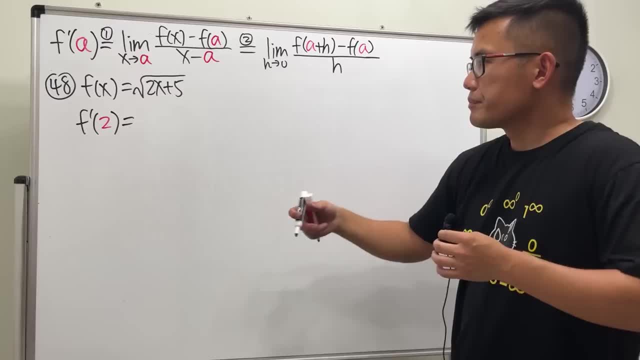 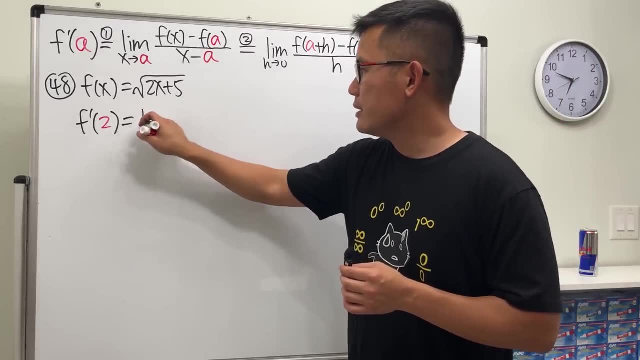 I think it's more straightforward, More direct this way, But this one also works. Don't worry, We will have a chance to practice this data, You will see. Anyway, this is the limit. Let's say that x is approaching 2.. 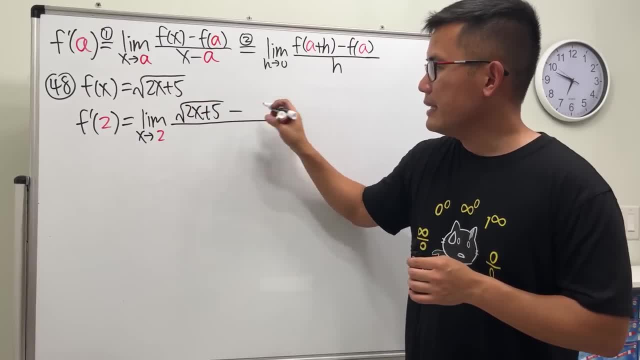 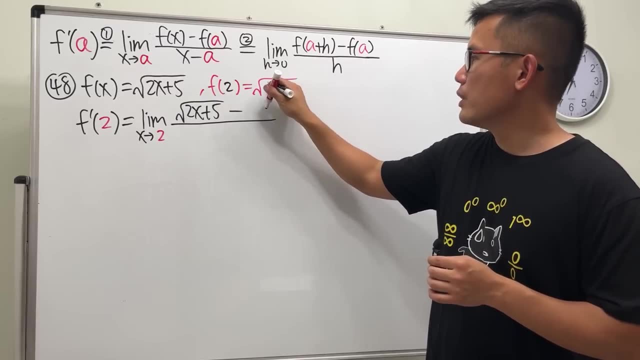 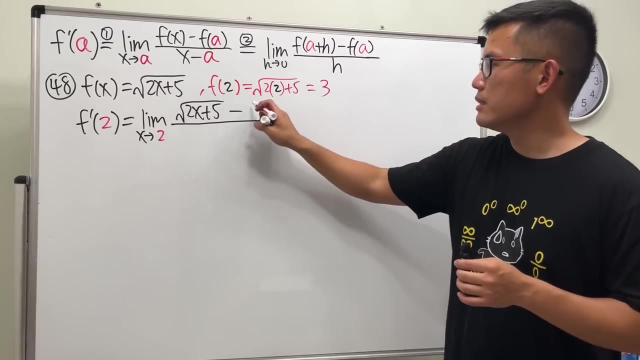 And then here we have our function: Square root of 2x plus 5 minus. Okay, We need the f of 2.. So let me write it down here: f of 2 equals square root of 2 times that 2, and then plus 5.. 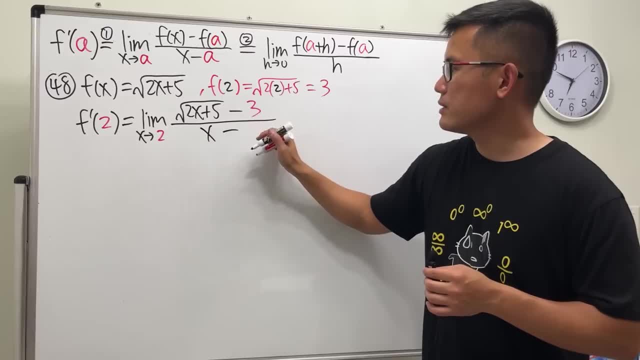 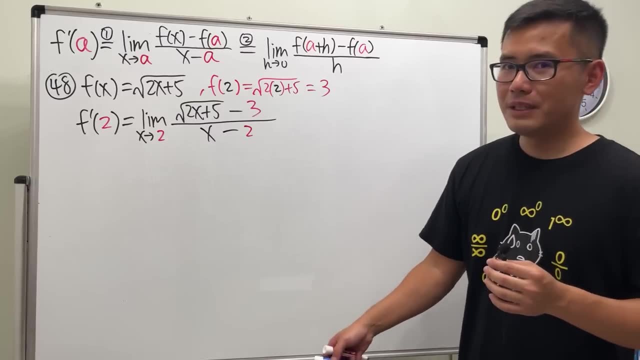 That's 9.. Take the square root, It's 3.. So 3 right here, And then over x minus 2.. Aha, Once we set this up, What's that called? It becomes that algebraic limit question, right, So let's go ahead. 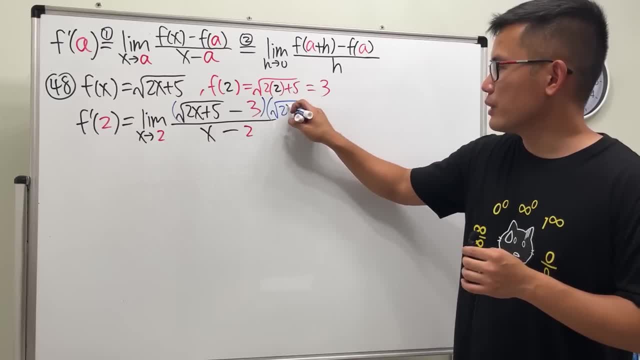 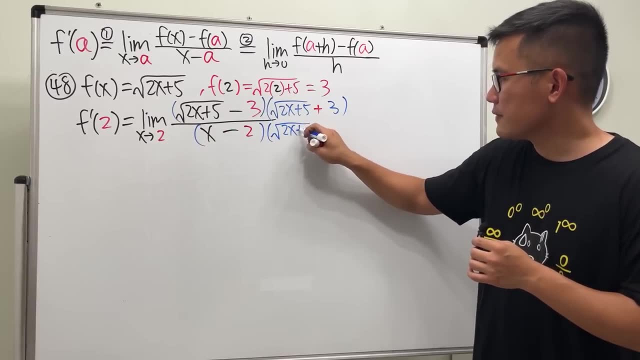 and just do the count. you get. Multiply the top and bottom by square root of 2x plus 5 plus 3.. And then let's also do the same on the bottom Square root of 2x plus 5 plus 3.. Okay, 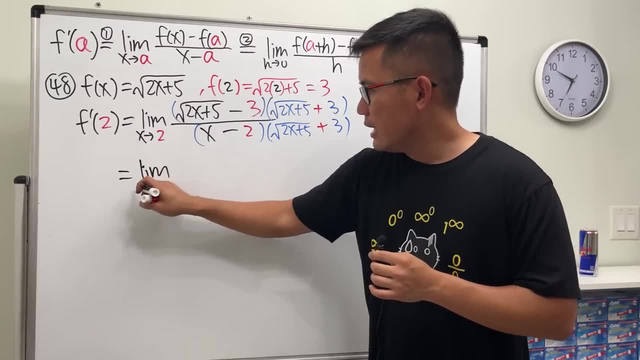 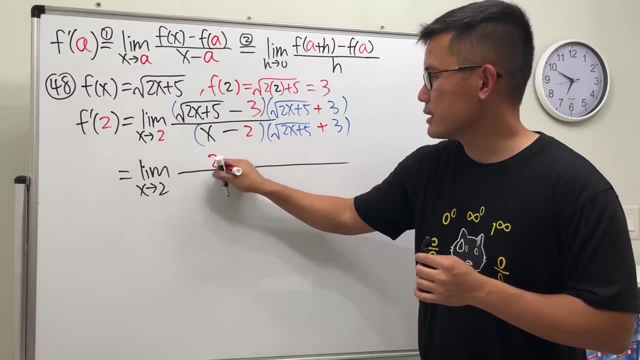 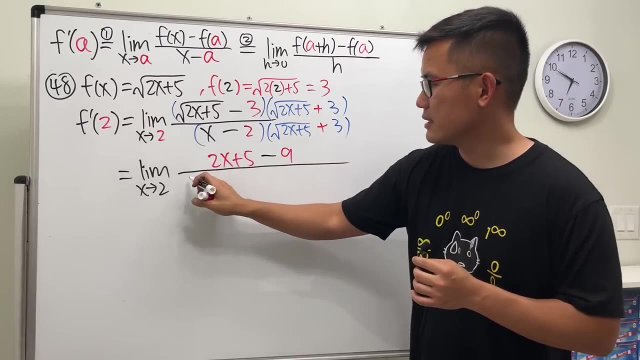 Now this is the limit as x approaching 2.. Okay, Square this. So we just have to multiply 2x plus 5 and then minus 3 times, So 3 squared, which is 9.. And then the bottom stays. 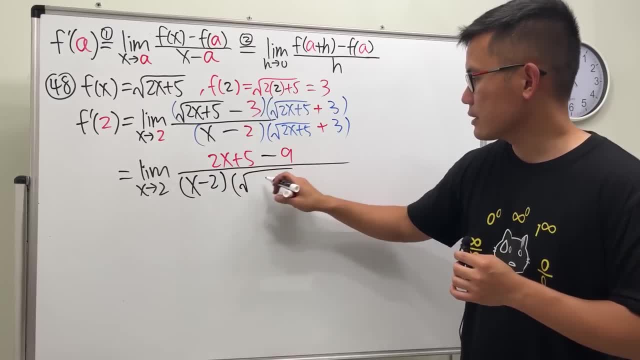 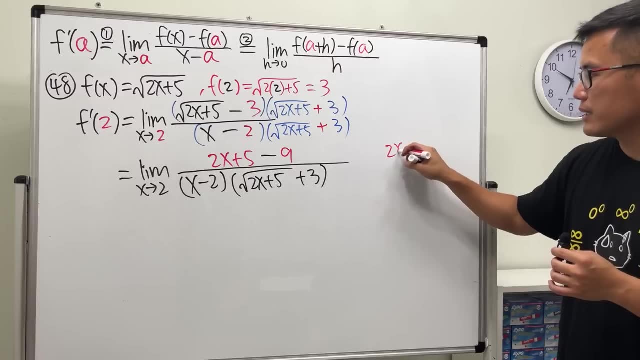 So x minus 2 times all that. Alright, The top right here, Let's just do it on the side real quick. That's 2x minus 4. And then we can factor out a 2, right? So it's this. 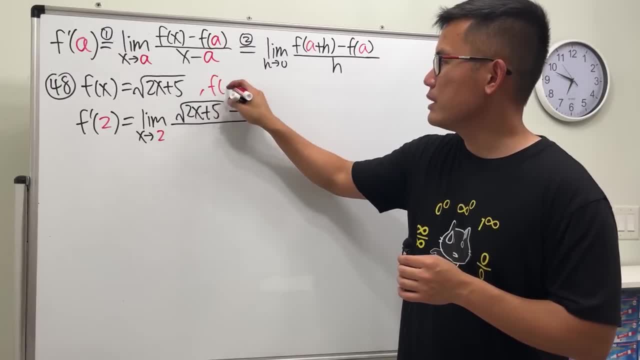 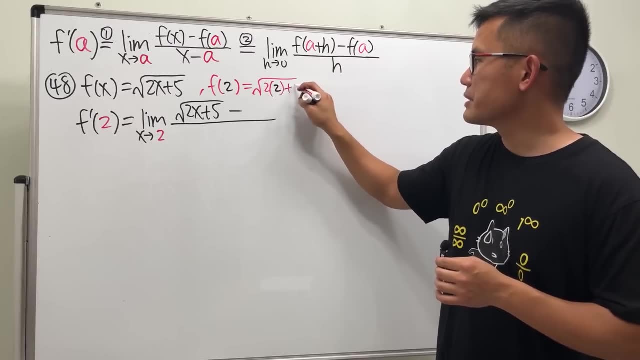 minus. okay, we need the f of 2, so let me write it down here: f of 2 equals square root of 2 times that 2 and then plus 5, that's 9. take the square root is 3, so 3, right here. 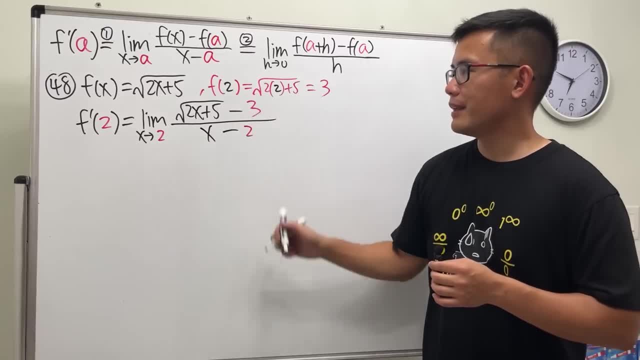 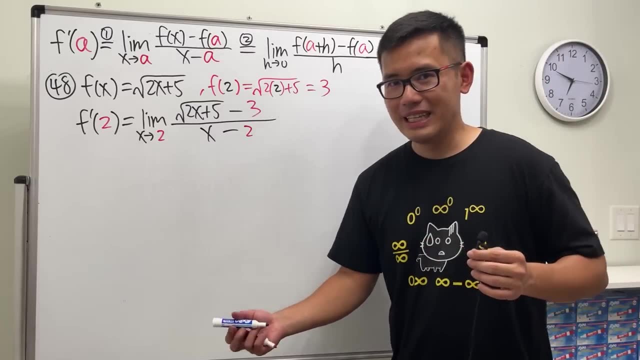 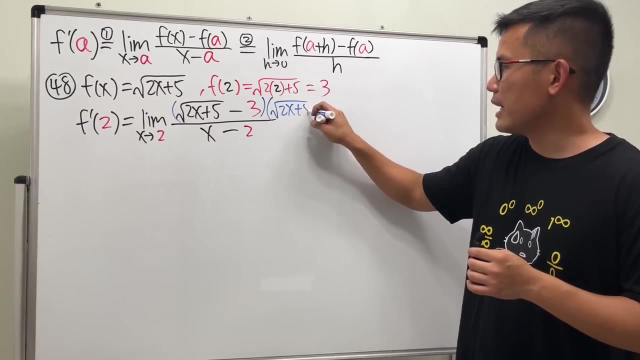 and then over x minus 2.. aha, once we set this up, it becomes what's that called? it becomes that algebraic limit question, right? so let's go ahead and just do the count you get: multiply the top and bottom by square root of 2x plus 5 plus 3, and then let's 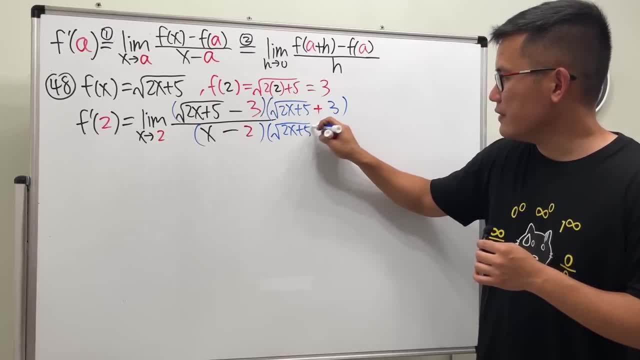 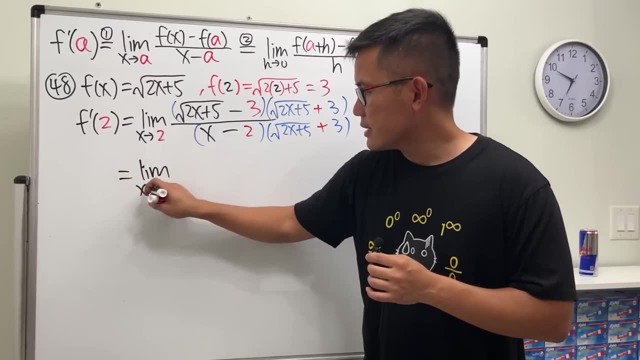 also do the same on the bottom square root of 2x plus 5 plus 3. okay, now this is the limit as x approaching 2.. okay, square this so we just have 2x plus 5 and then minus 3 times 3. square, which is 9, and then minus 3, square which is 9, and then minus 7 plus 5.. 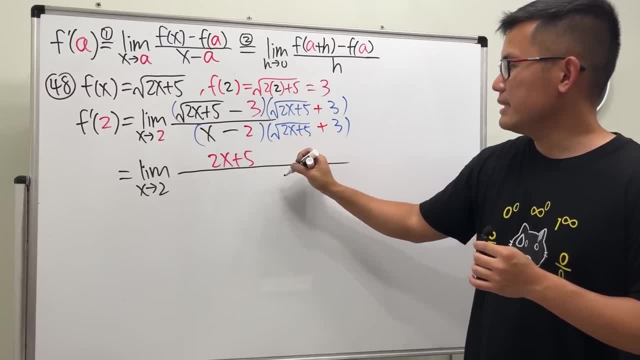 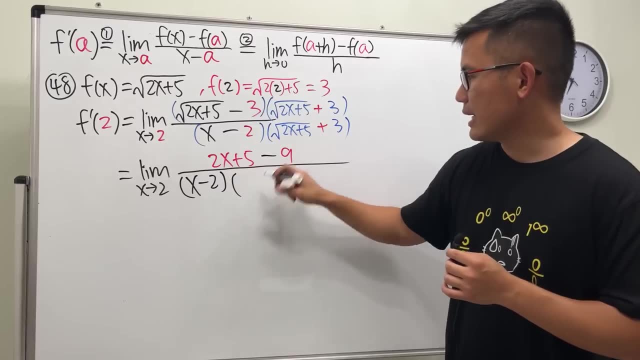 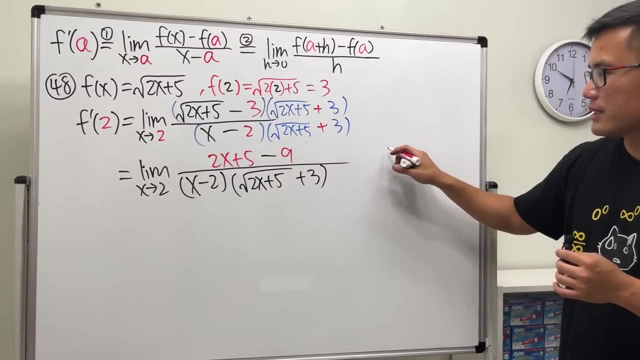 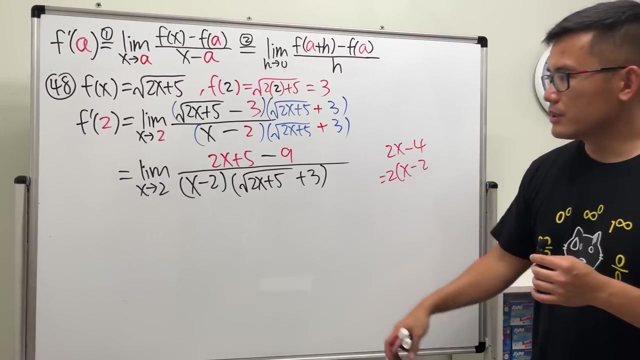 So we just have 2x plus 5 and then minus three times three square, which is nine, and then minus six. the bottom stays. so x minus 2 times all that. all right, the top, right here. let's just do it on the side real quick. that's 2x minus 4, and then we can factor out a 2, right, so it's this. so i'm just 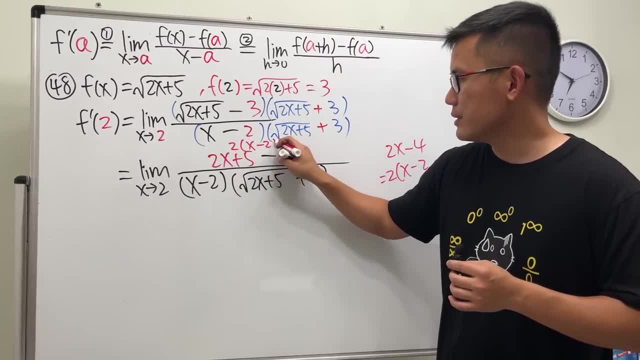 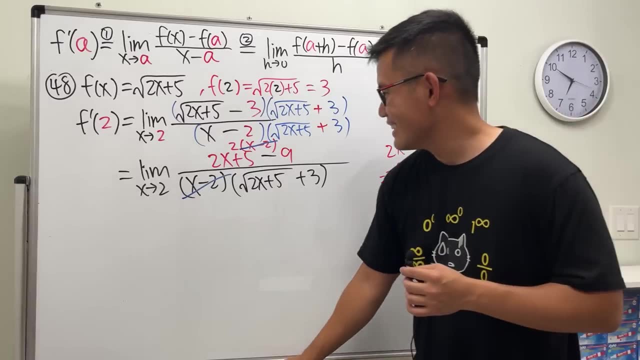 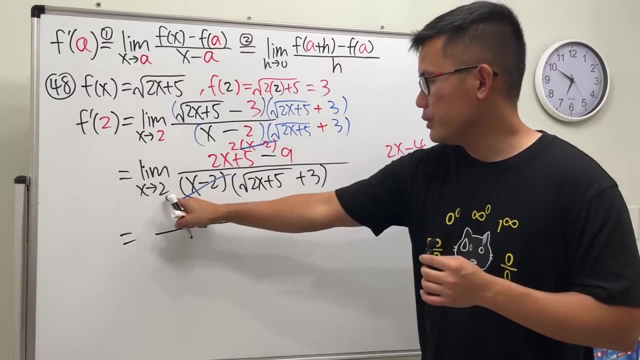 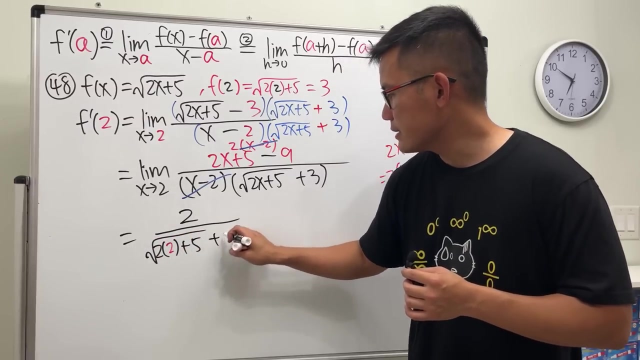 going to squeeze out the result here: 2 times x minus 2, okay, and then i'm just going to cancel the x minus 2. x minus 2, perfect, all right, we have this 2 right here, though be really careful. so 2 over. put this 2 in here. so we have square root of 2 times 2 plus 5 and then plus 3. 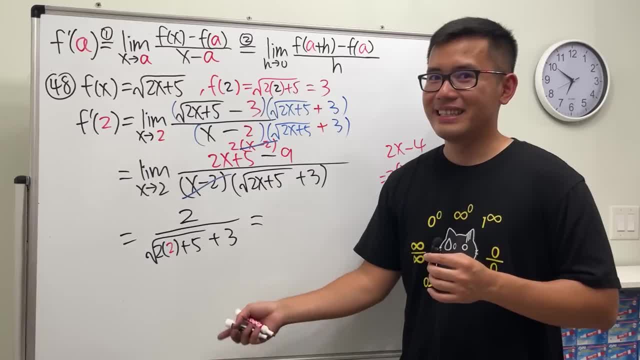 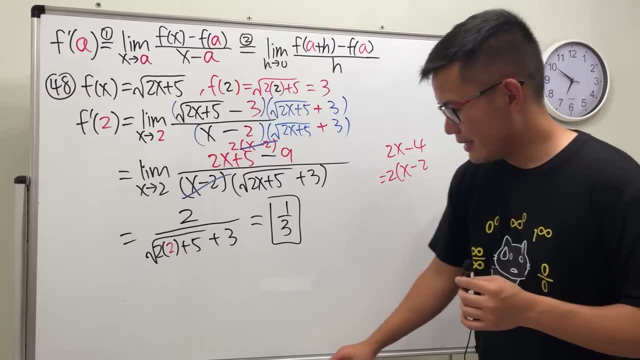 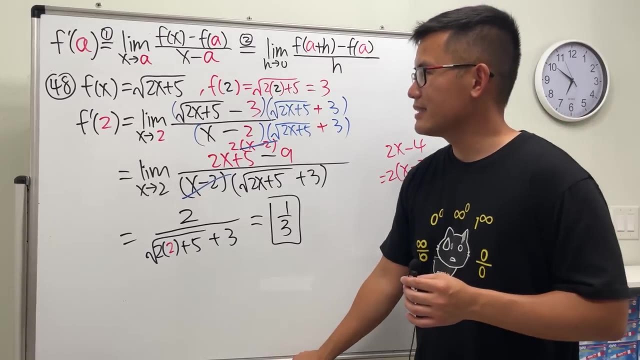 that's 9. square root of 9 is 3, 3 plus 3 is 6, 2 over 6 is 1, 3.. is it? yeah, okay, all right, so now, then? let's. yeah, that's okay, let's just do this with actual numbers. uh, for the derivative, for the. 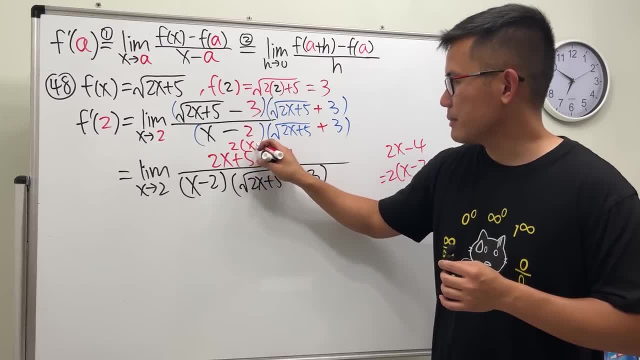 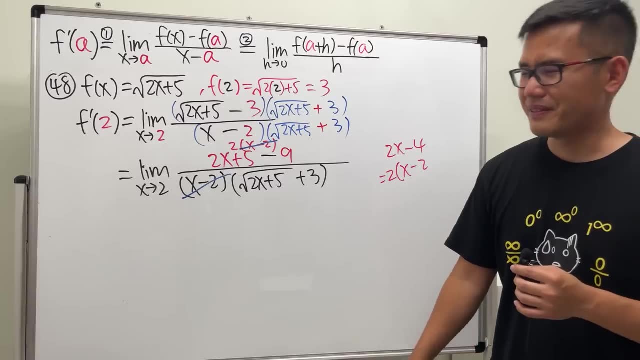 So I'm just going to squeeze out the result here: 2 times x minus 2.. Okay, And then I'm just going to cancel the x minus 2.. Perfect, Alright, We have this 2 right here, though, Be really careful. 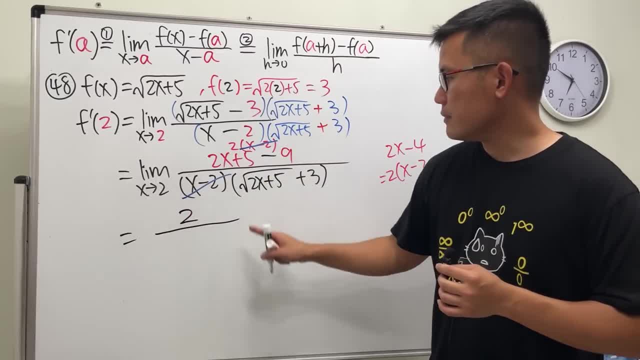 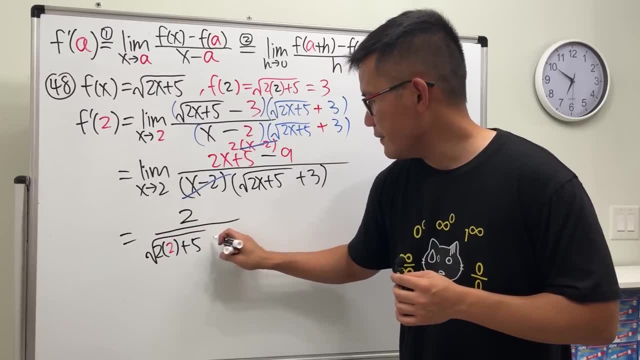 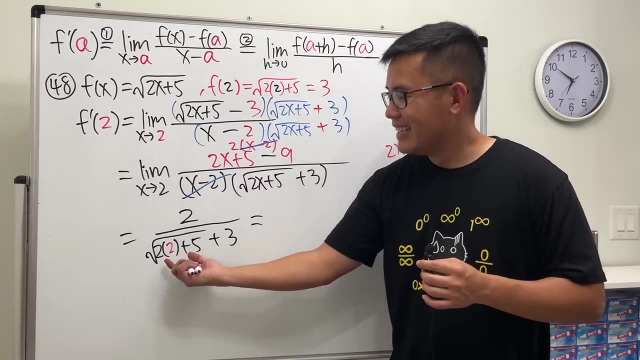 So 2 over. Put this 2 in here. So we have square root of 2 times 2 plus 5 and then plus 3.. That's 9.. Square root of 9 is 3.. Plus 3 is 6.. 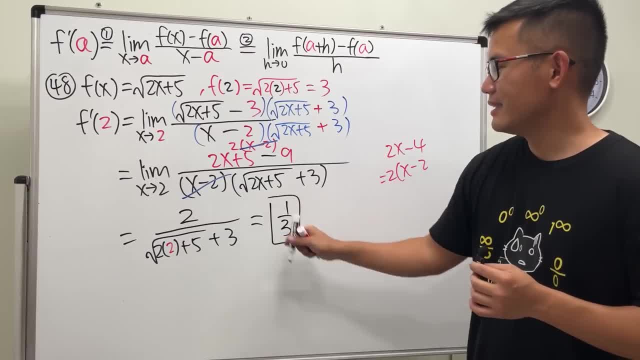 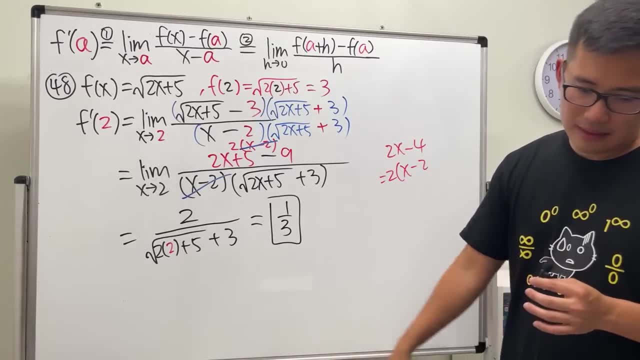 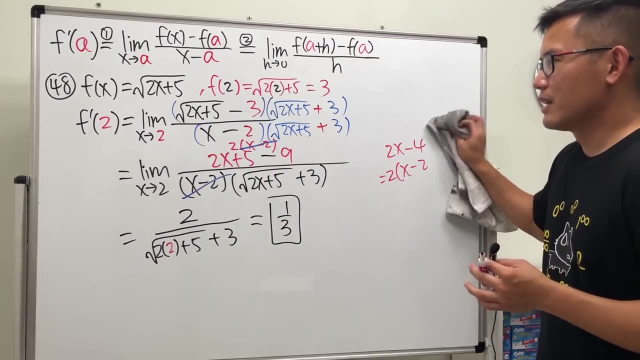 2 over 6 is 1. third, Is it? Yeah, Okay, Alright, It's enough. Then let's. Yeah, that's okay, Let's just do this with actual numbers For the derivative, for the derivative technique. it's coming anyway, So don't worry. 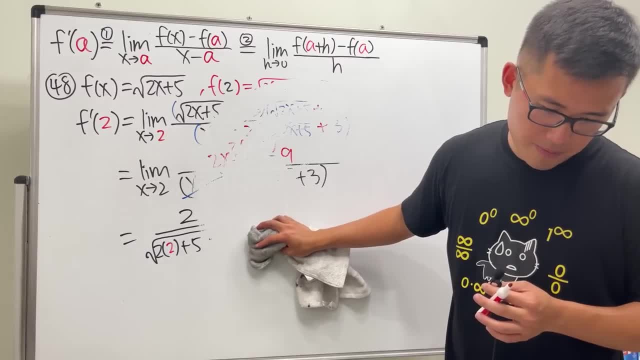 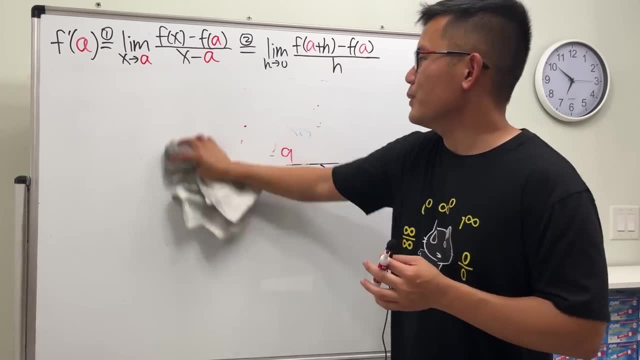 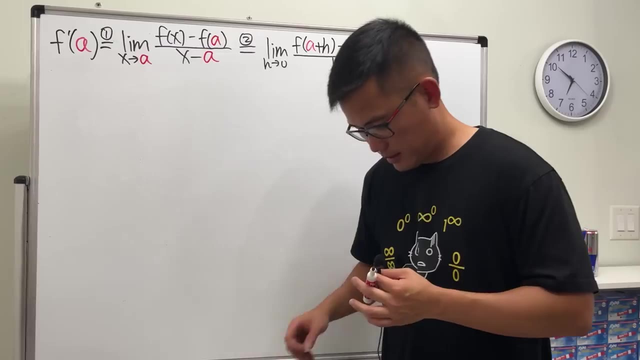 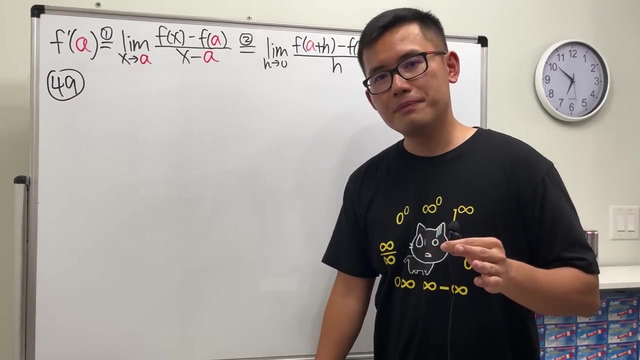 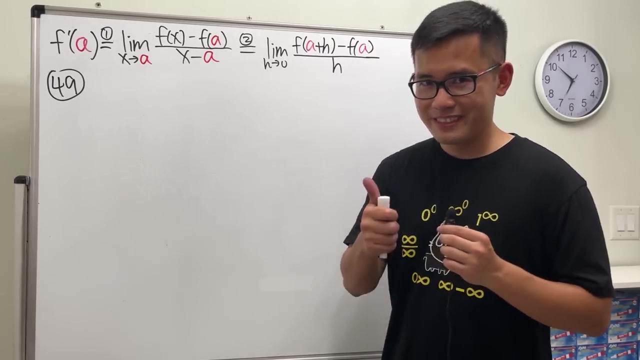 Let's practice. We have 2 more questions. Okay, anyway, though. 50- What am I talking about? Number 49.. If you are still watching, leave your timestamp right now, Appreciate it. You're working hard, I'm working hard too. 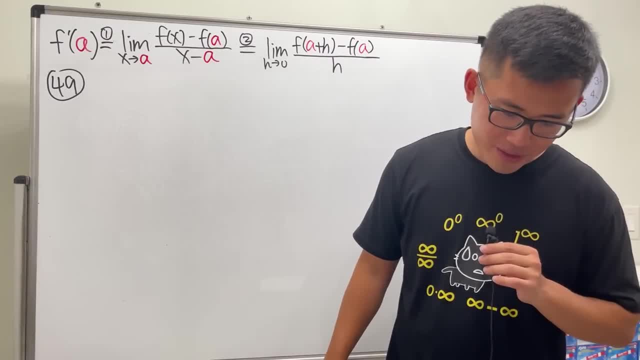 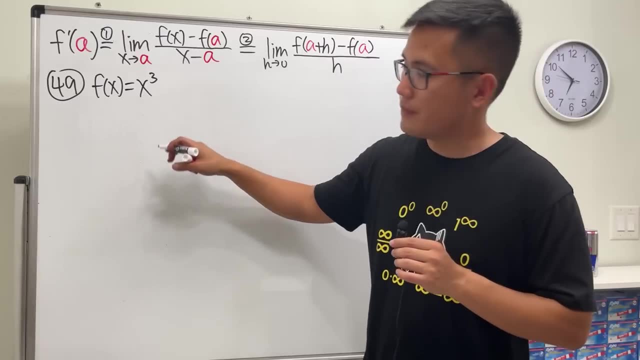 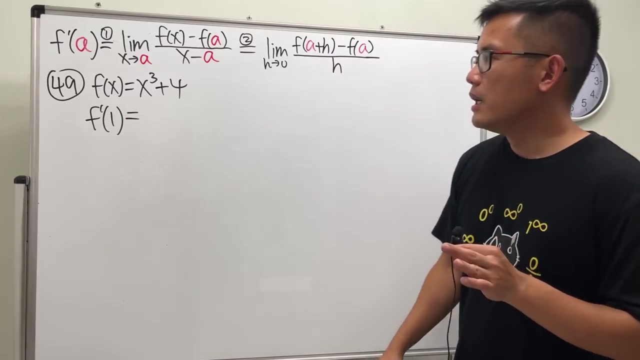 Okay, Let's see Number 49.. F of x equals x to the third power, plus 4.. And then we want f prime of 1.. So I'll use the power rule for this later on, But anyway, though, if we want f prime, 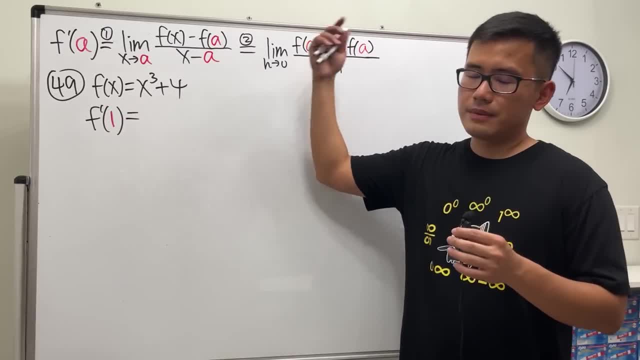 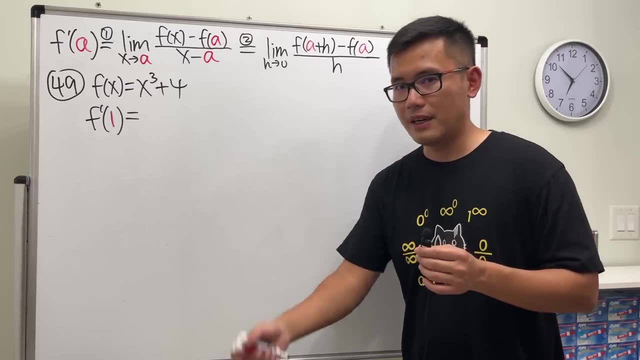 of 1,, as I mentioned here a couple minutes ago or so. if you use this definition, it's easier to you will have to factor it If you like factoring, And if you use this, then you will have to expand it. 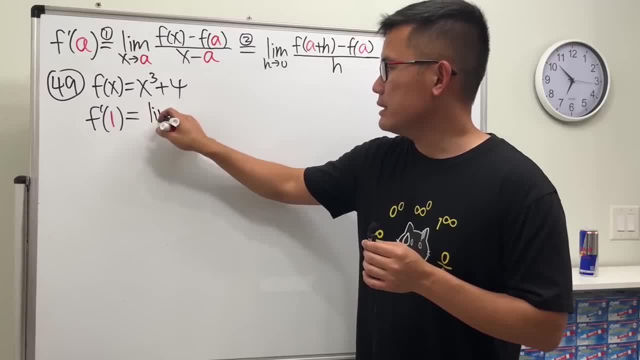 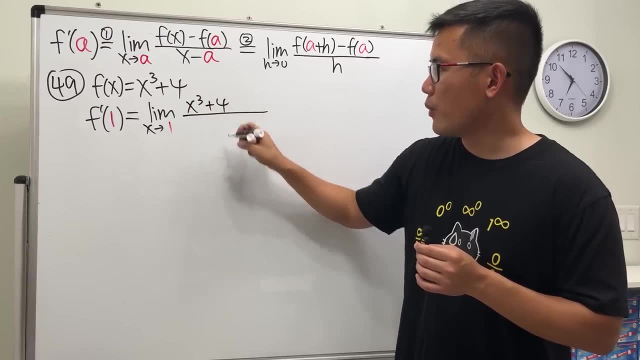 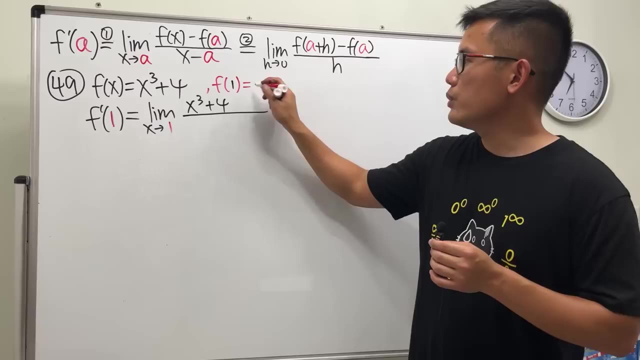 Let's just do this one. So this, right here, is the limit, as x approaching 1 function is x to the third power plus 4.. And then we need to know the f of 1, right, So f of 1 is just equal to. 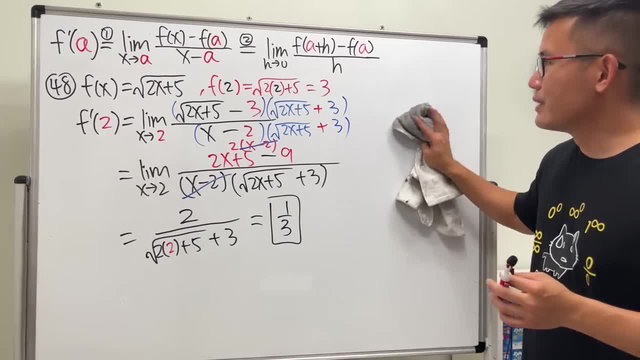 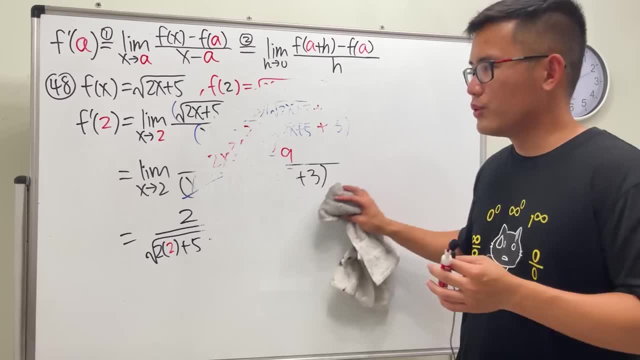 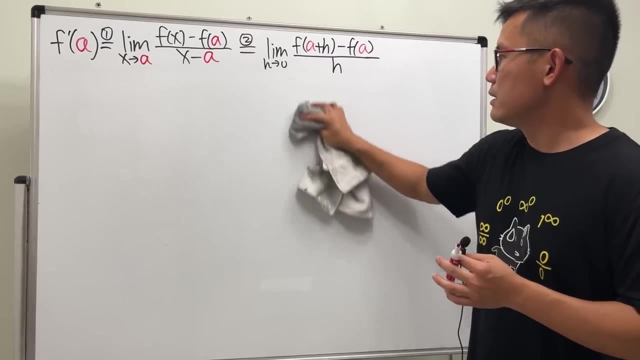 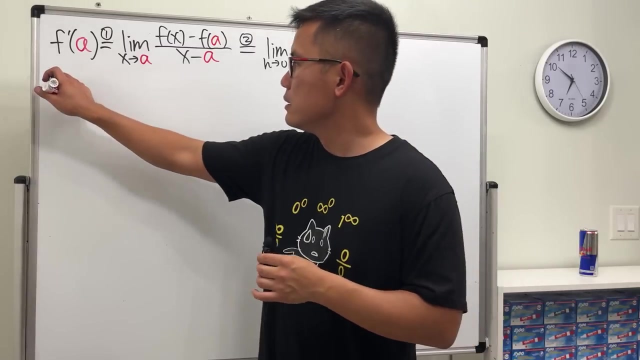 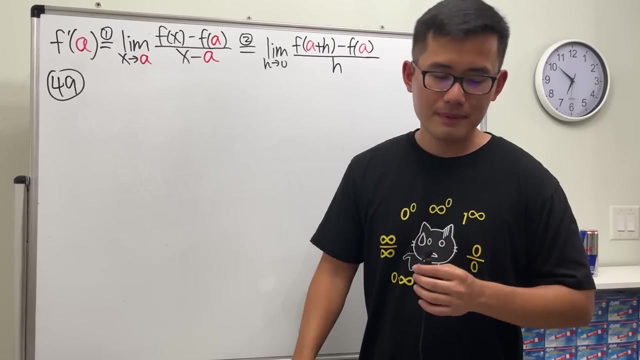 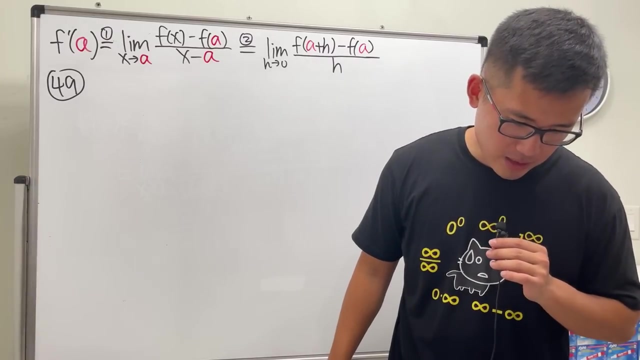 uh, derivative technique. uh, it's coming anyway, so don't worry, let's practice. oh, we've got two more questions. okay, anyway, though, 50. that's number 49. if you are still watching, leave your time stamp right now. appreciate it, you're working hard. i am working hard too. okay, let's see number 49. 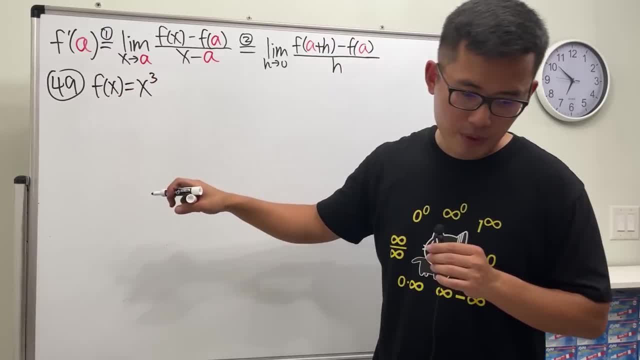 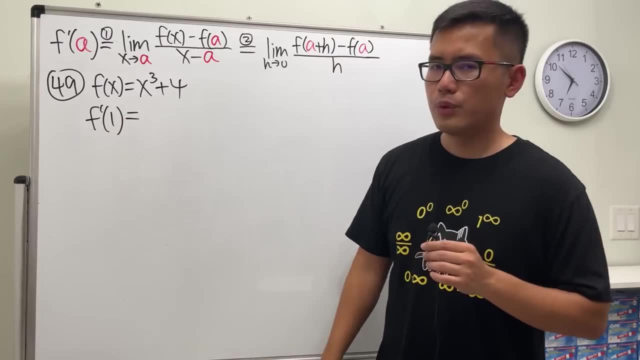 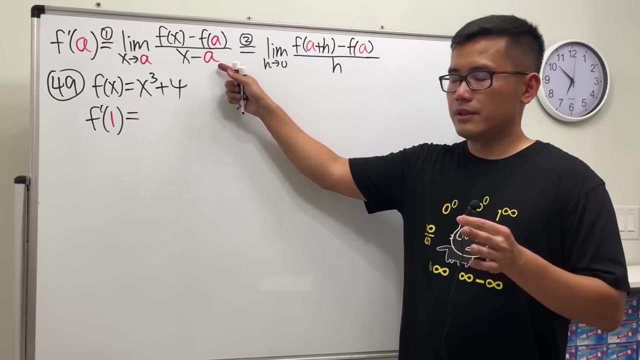 f of x equals x to the third power plus four, and then we want f prime of one, so use the power rule for this later on. but anyway, though, if we want f prime of one- as i mentioned here a couple minutes ago or so- if you use this definition, it's easier to- you will have to factor. 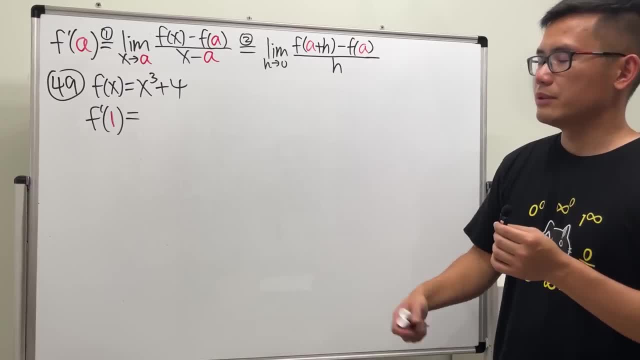 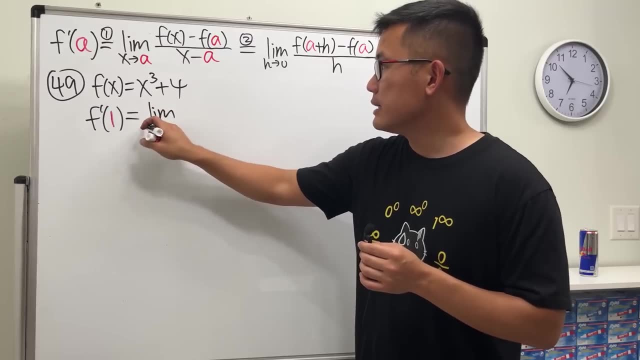 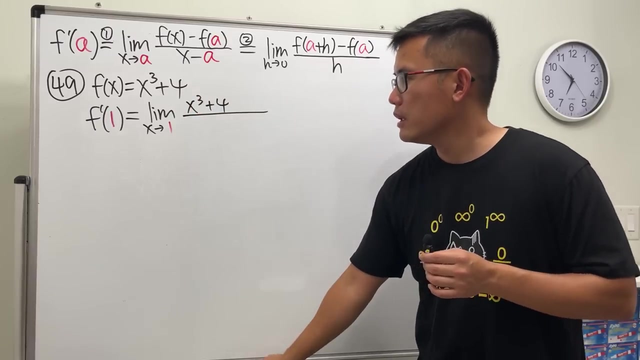 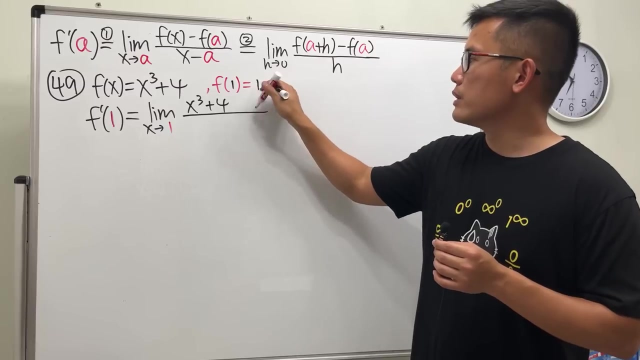 it. if you like factoring, and if you use this, then you will have to expand it. now let's just do this one. so this right here is the limit, as x approaching one function is x to the third power plus four. and then we need to know the f of one, right, so f of one is just equal to one to the third power. 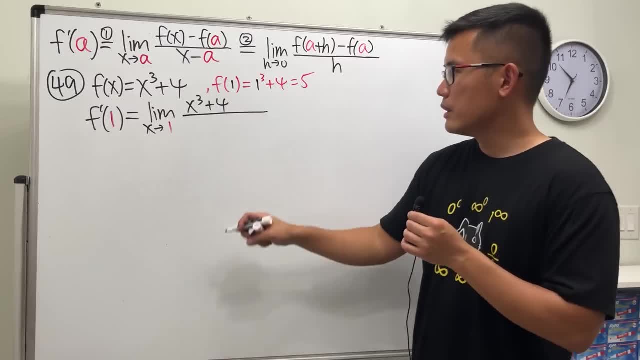 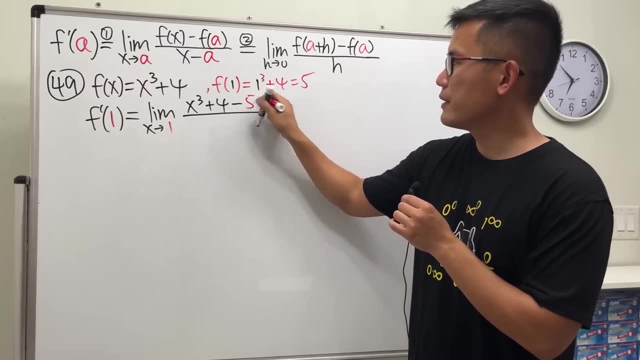 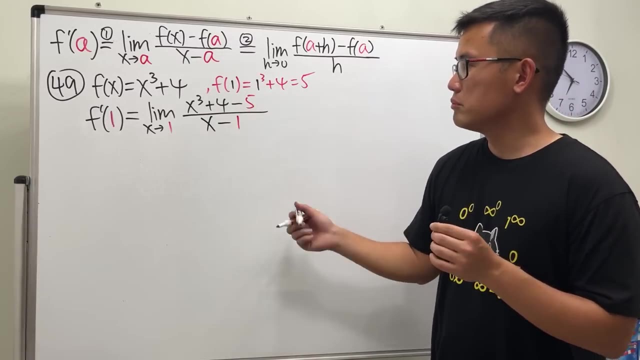 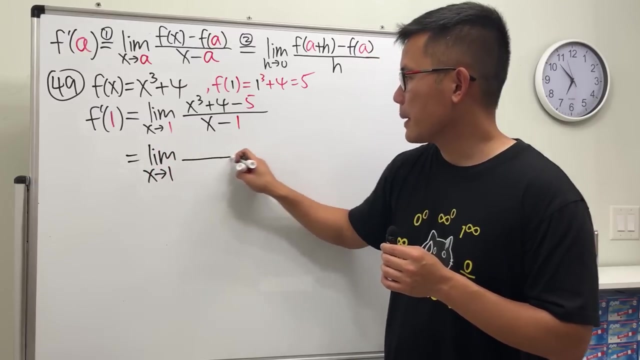 plus four, which is five. so this means we have x plus third power plus four, and then minus five f. yeah, and then on the bottom we have x minus one. yeah, it's not bad to factor this at all, so this is good. limit x approaching one on the top is just x to the third power minus one, and on the bottom 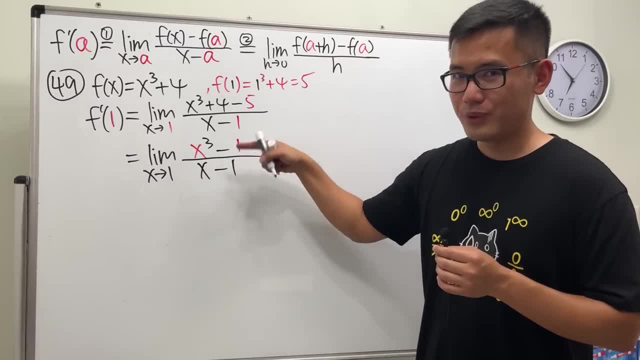 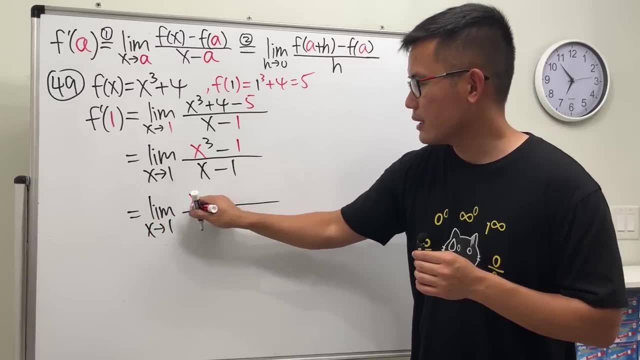 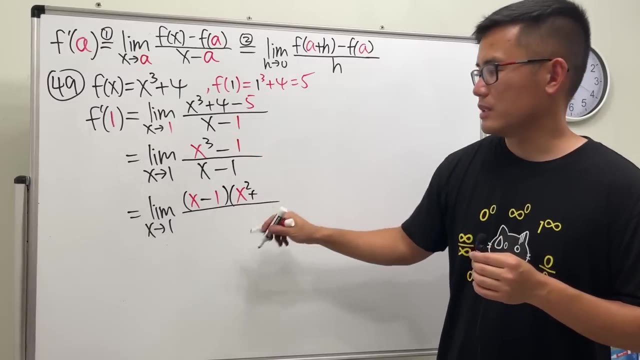 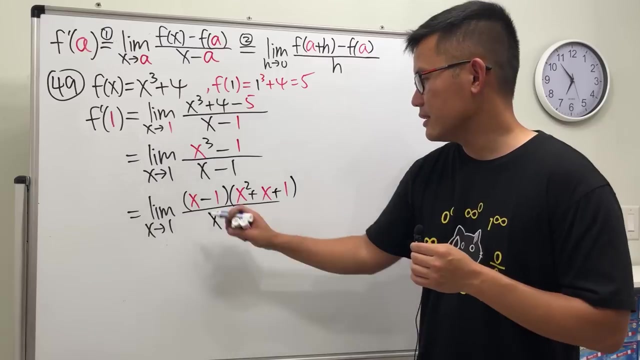 is x minus one. okay, this is the same as one to the third power. so factor it difference of two cubes. here's two cubed and four cubed. both are equal. so we get x minus one. we get x minus one times x squared plus one times x, which is just x, and then plus one, squared which. 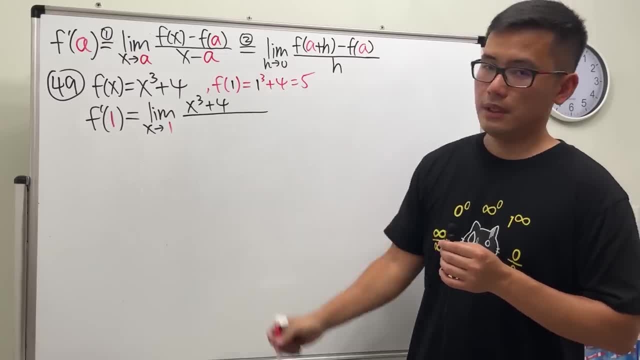 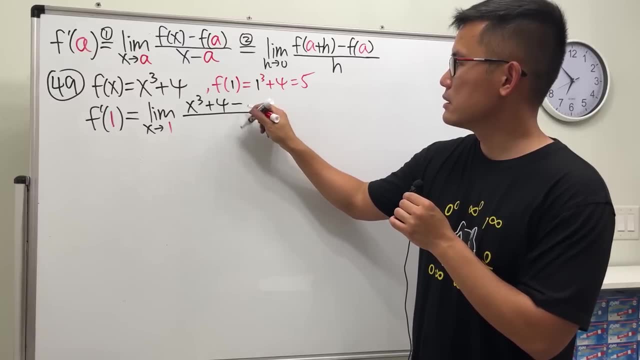 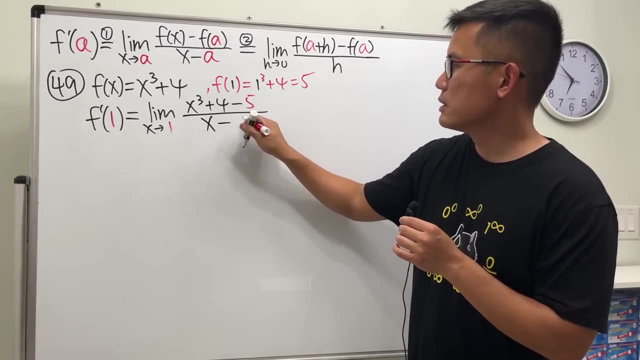 1 to the third power plus 4, which is 5.. So this means we have x to the third power plus 4 and then minus 5.. Yeah, And then on the bottom we have x minus 1.. Yeah, It's not bad to factor this at all. 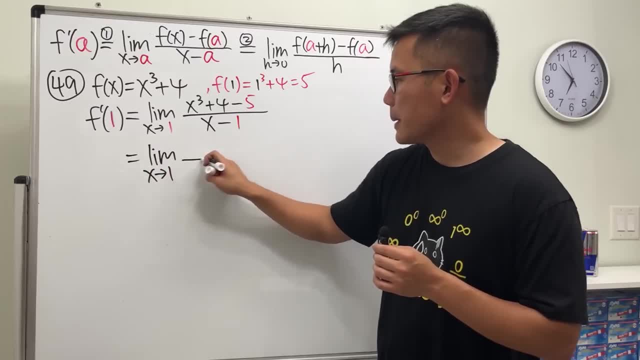 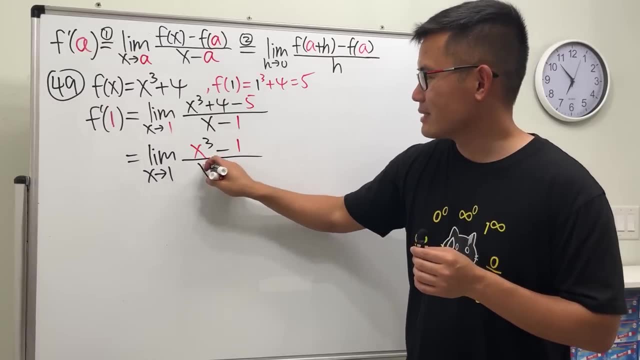 So this is good. Limit: x approaching 1.. On the top is just x to the third power minus 1.. And on the bottom is x minus 1.. Okay, This is the same as 1 to the third power. So factor it. 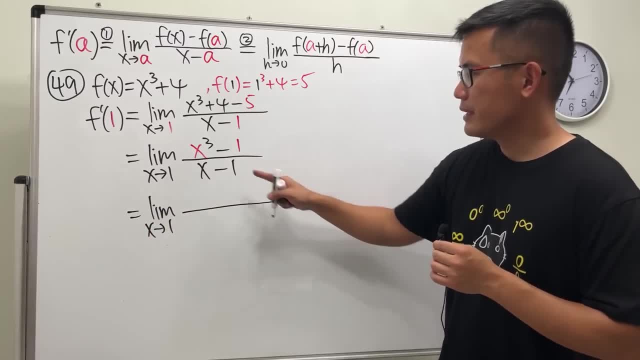 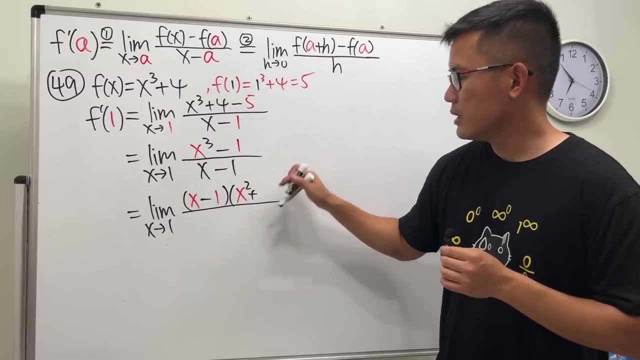 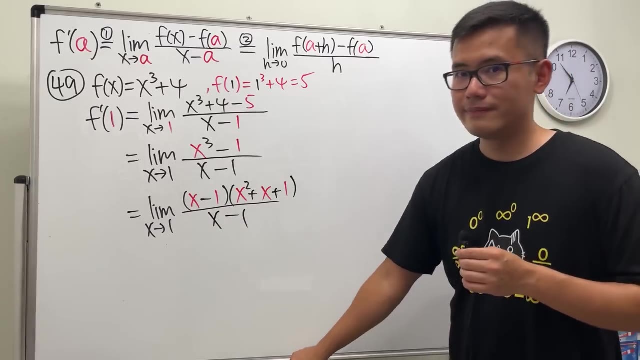 Difference of 2 cubes. We get x minus 1 times x squared, plus 1 times x, which is just x, And then plus 1 squared, which is just 1.. And then on the bottom is x minus 1.. And then x minus 1. 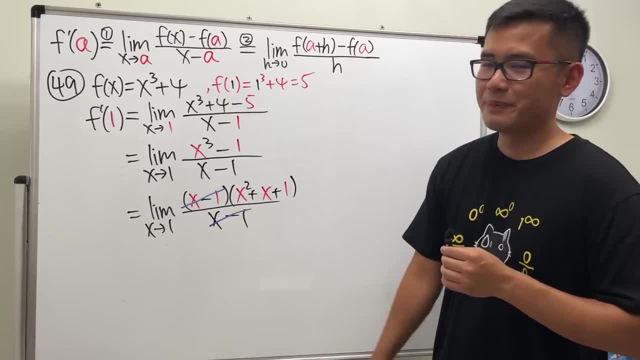 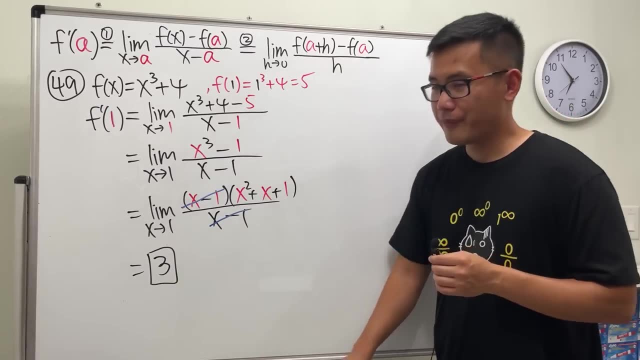 cancel. Ladies and gentlemen, put a 1 here, here. 1 plus 1 plus 1. We get 3.. Yay, Cool. Now let's see if we can finish this equation in 3 seconds. No like, let's. 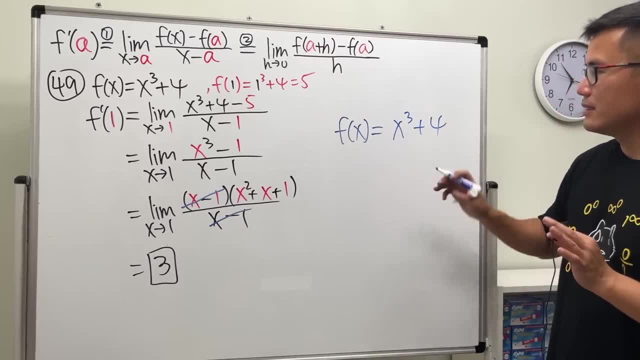 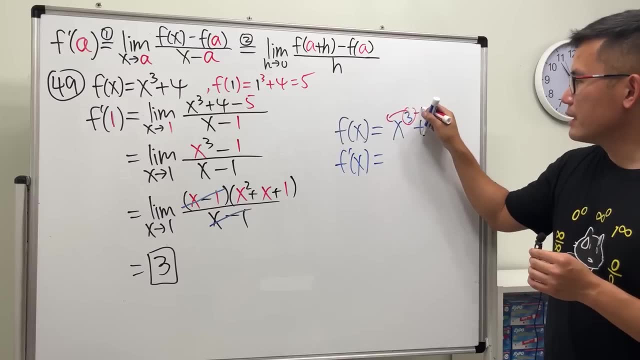 5 seconds. I'm copying the equation, so it doesn't count. Ready, Okay, f. prime of x. bring the power to the front minus 1.. We get 3x squared. Well, this is just a 4.. But if you use 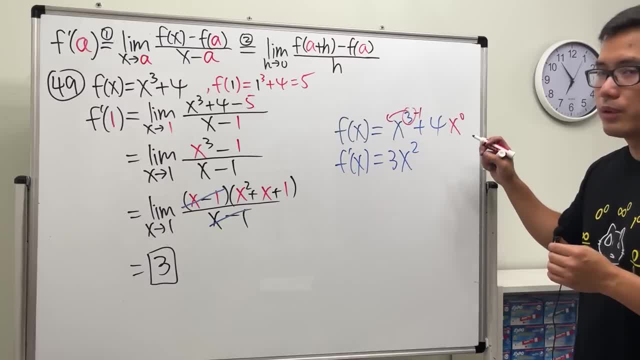 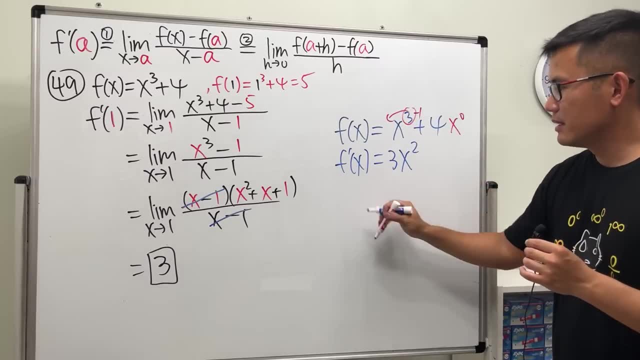 the power rule. you can look at this as x to the zero's power. put a 0 to the front. 0 times 4 is 0. So it's no more. So we just have this f prime of 1, 3 times 1 squared. 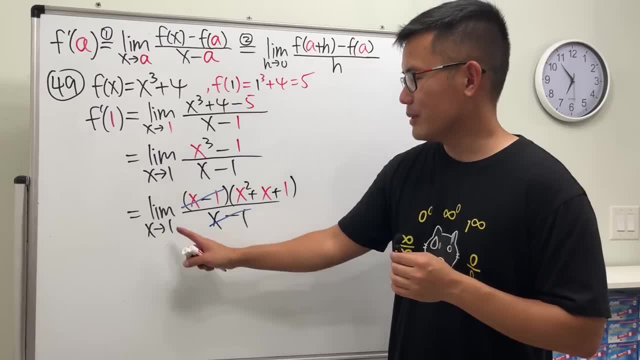 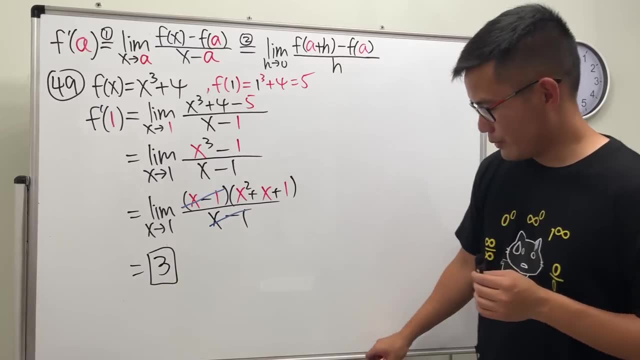 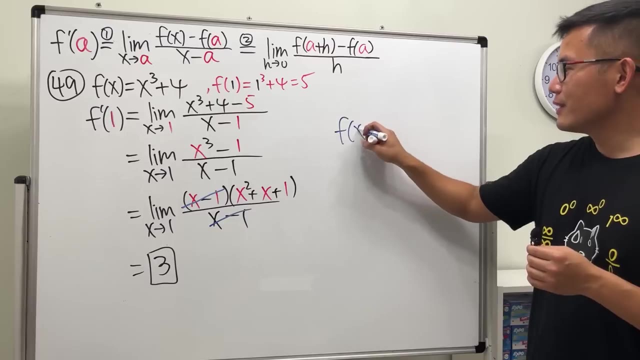 is just one and then on the bottom is x minus one and then x minus one. cancel, ladies and gentlemen, put a one here here, one plus one plus one, because three, yay, cool, see if we can finish this questions in three seconds. no, like that's five seconds. I'm copying another question also, isn't? it doesn't count, ready, okay? 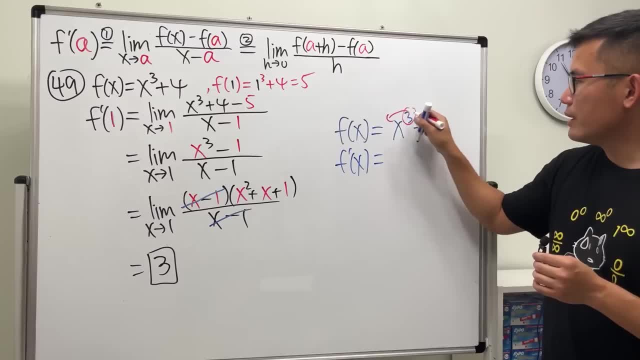 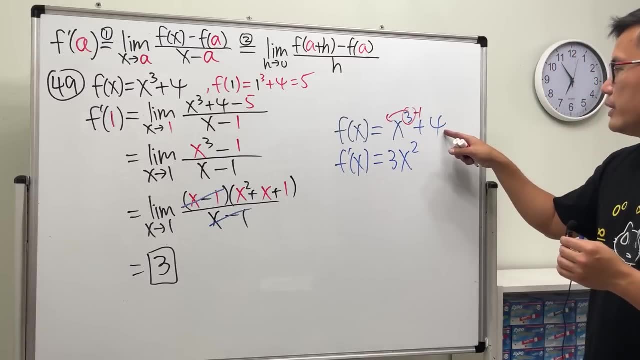 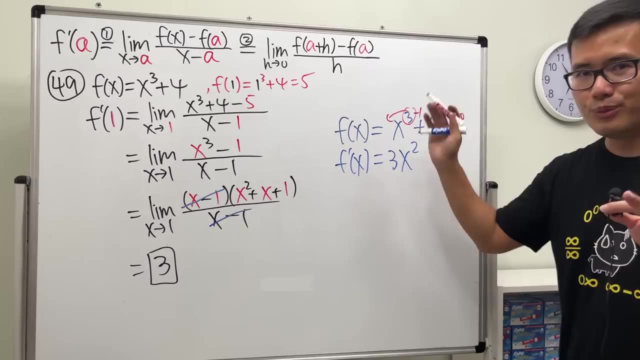 f: prime of X. bring the power to the front minus 1, we get 3x square. well, this is just a 4, but if you use the power rule you can look at this as X to the zeros power. put us through to the front: 0 times 4 is 0, so it's no more. so we just 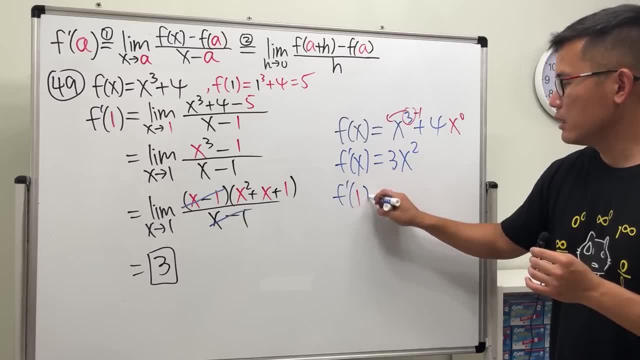 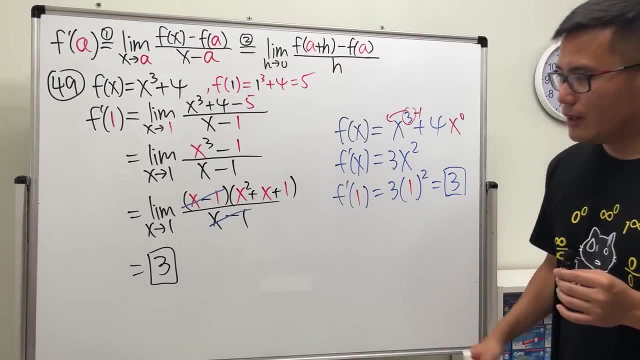 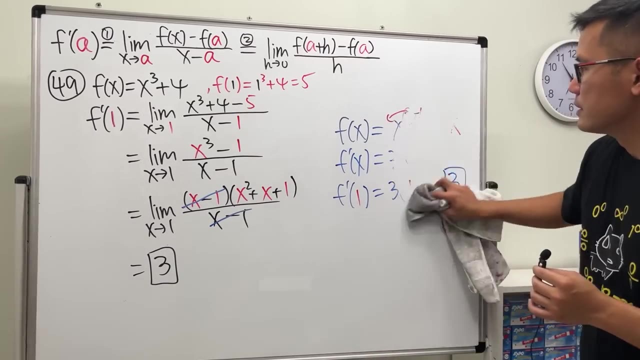 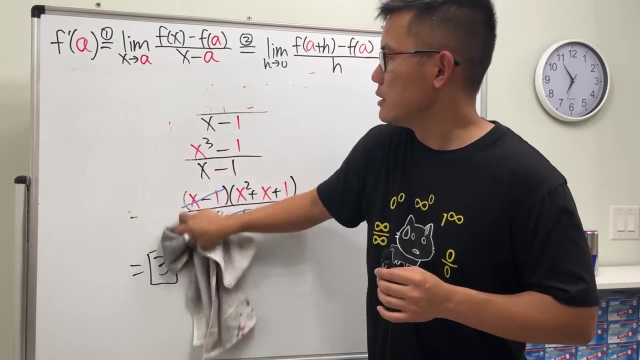 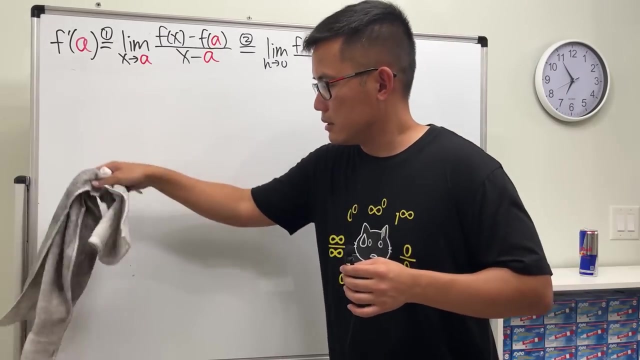 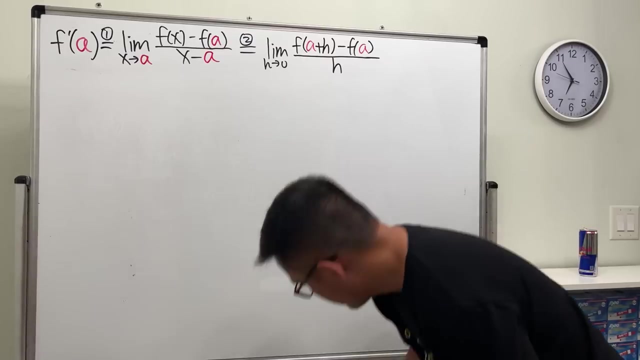 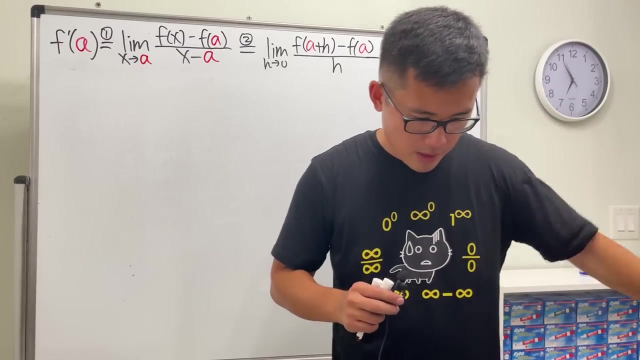 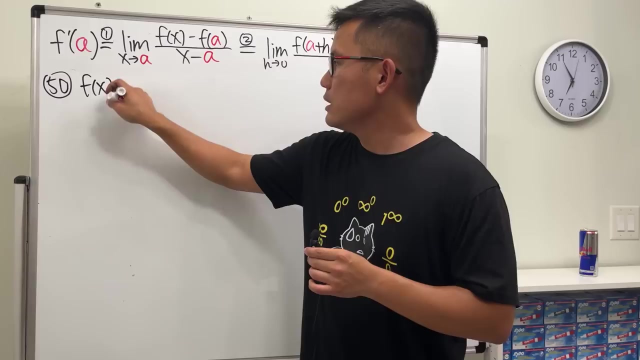 have this f prime of 1, 3 times 1 square and we get 3. Wow, powerful, power rule, so powerful, isn't it okay? well, alright, number 50. here we have our alright number 50. here we have our alright number 50. here we have our function is just. 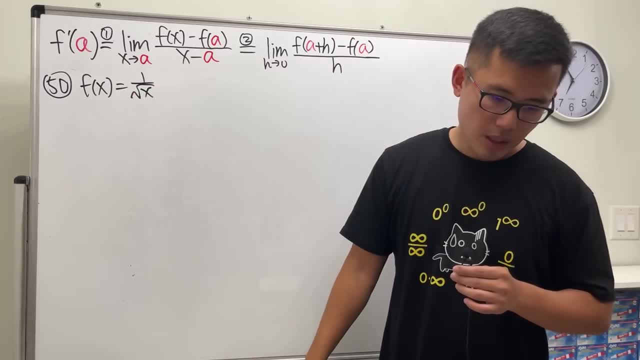 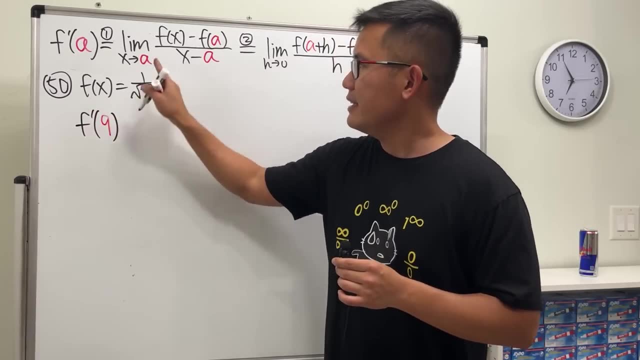 function is just. function is just 1 over square root of X, and we want f prime of 9. so here we go: 1 over square root of X and we want f prime of 9. so here we go: 1 over square root of X and we want f prime of 9. so here we go: f prime of 9. this is my 9. this is my a. 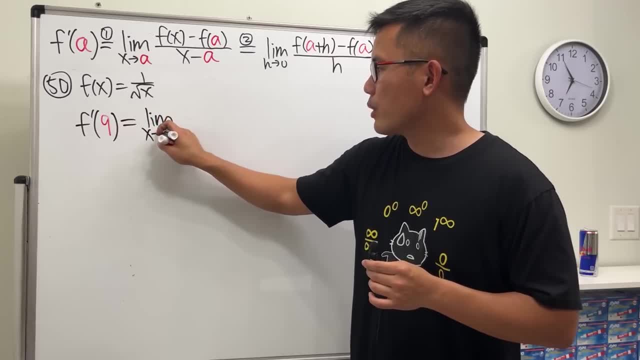 f prime of 9. this is my 9. this is my a f prime of 9. this is my 9. this is my a here we go- limit X approaching 9. our here we go: limit X approaching 9. our here we go- limit X approaching 9. our function is 1 over square root of X and. 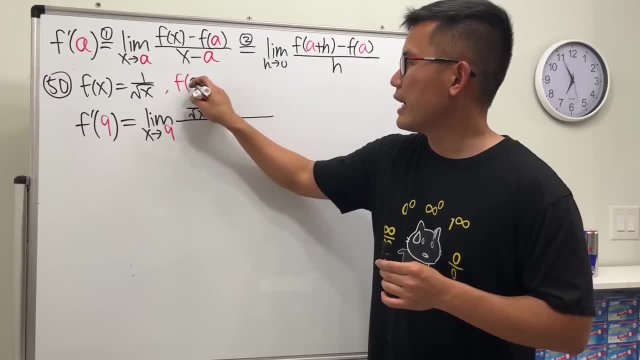 function is 1 over square root of X, and function is 1 over square root of X, and then we have to minus f of 9, which is. then we have to minus f of 9, which is. then we have to minus f of 9, which is just 1 over square root of 9, and that's. 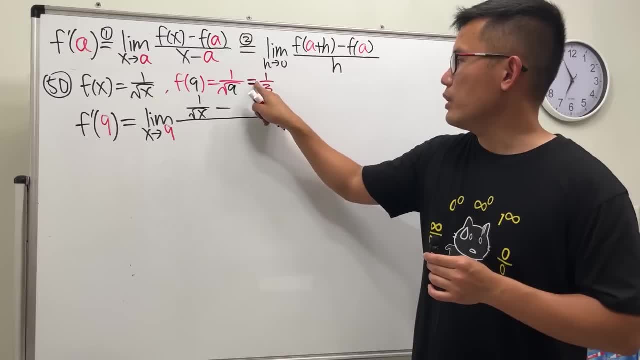 just 1 over square root of 9, and that's just 1 over square root of 9, and that's just 1 3rd. okay, not bad at all, so minus just 1 3rd. okay, not bad at all, so minus just 1 3rd. okay, not bad at all, so minus 1 3rd. 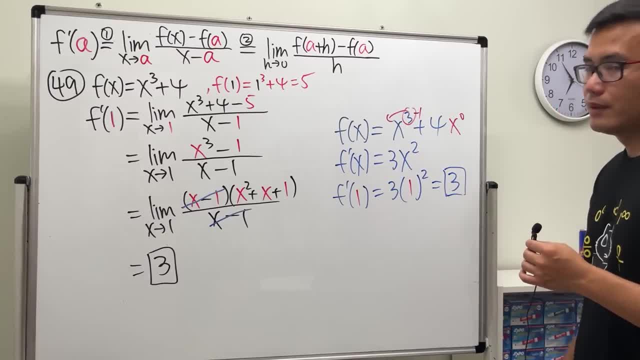 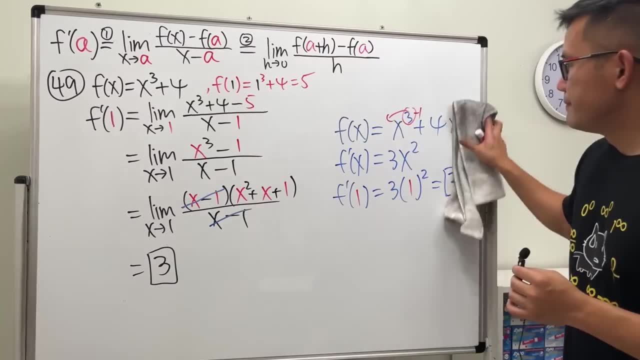 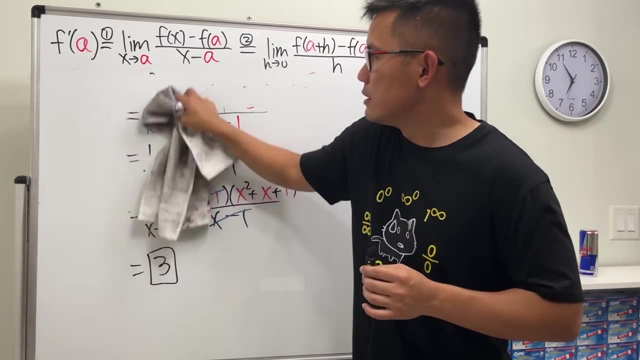 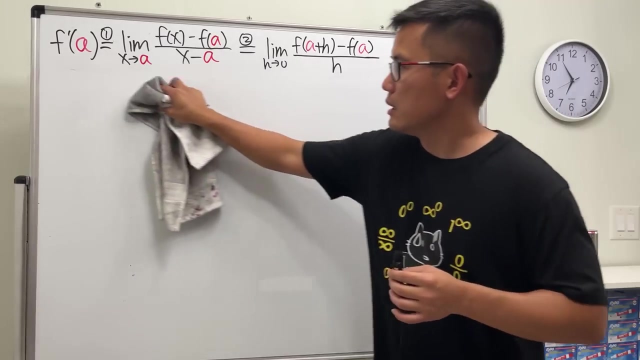 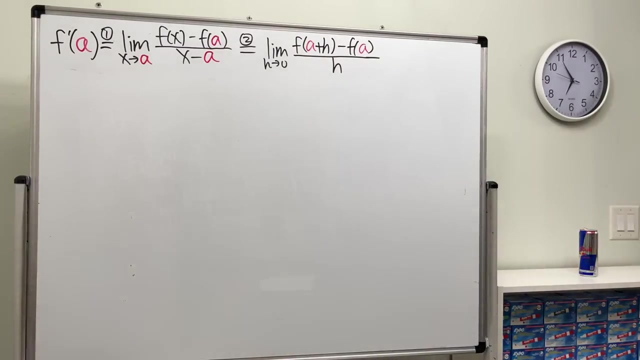 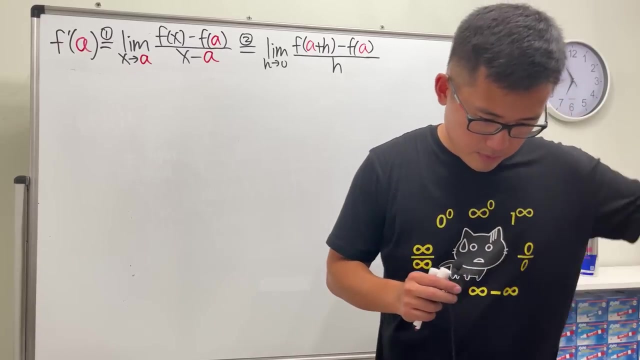 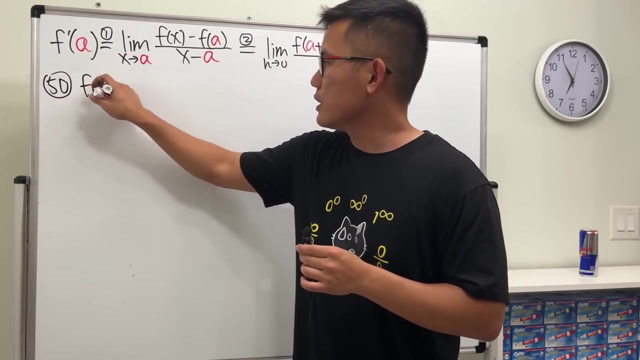 and we get 3.. Wow, Wow, Powerful Power rule. So powerful, isn't it? Okay, Alright, Number 50.. Here we have our function. It's just 1 over square root of x And we want f prime. 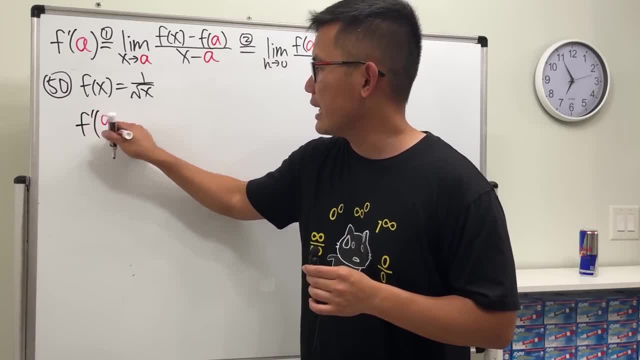 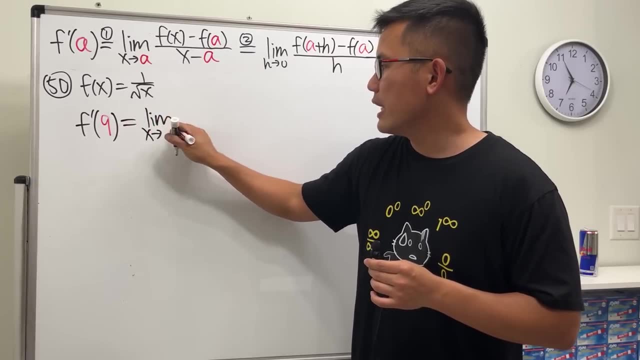 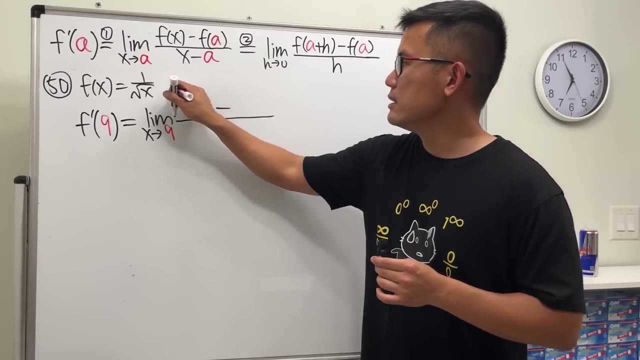 of 9.. So here we go. f: prime of 9.. This is my 9.. This is my a. Here we go. Limit x approaching 9.. Our function is 1 over square root of x And we have to minus. 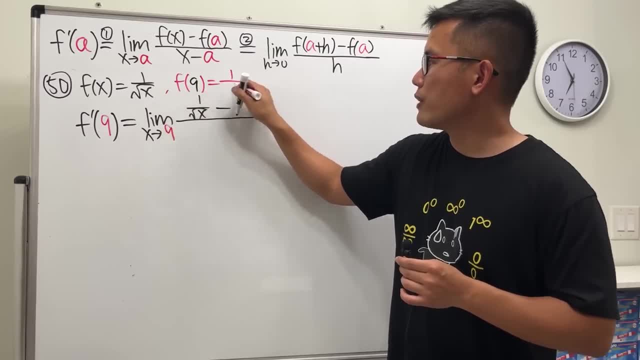 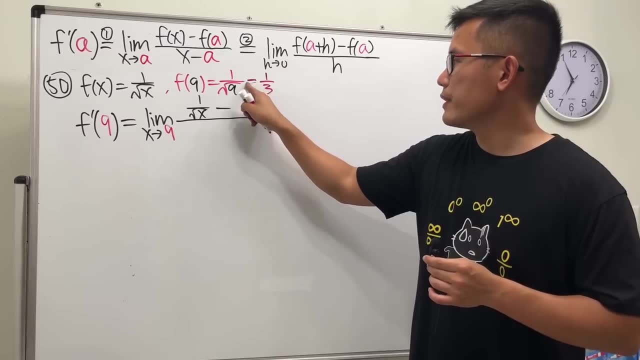 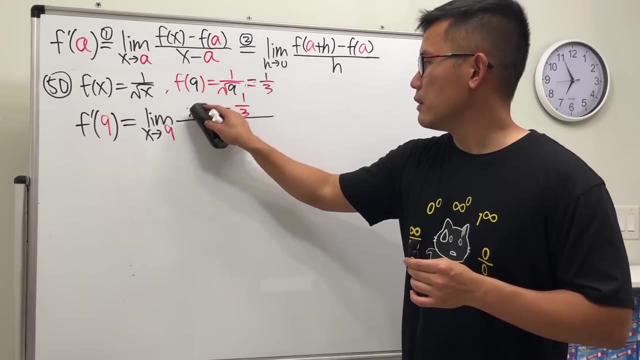 f of 9. Which is just 1 over square root of 9.. And that's just 1 third. Okay, Not bad at all, So minus 1 third. Let me just write it down. Let me just write it down. 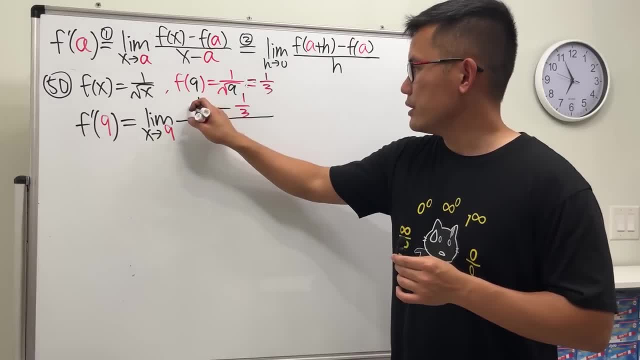 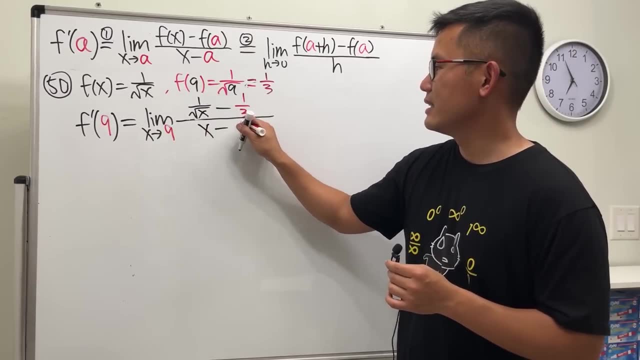 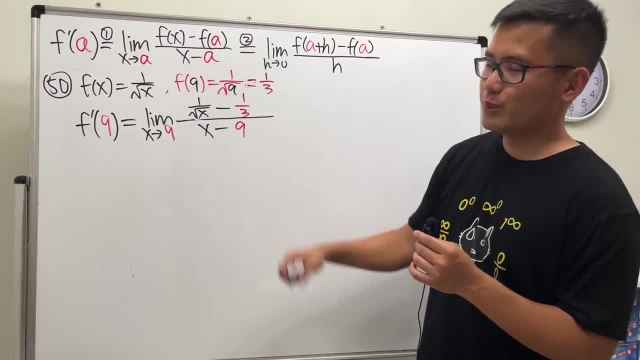 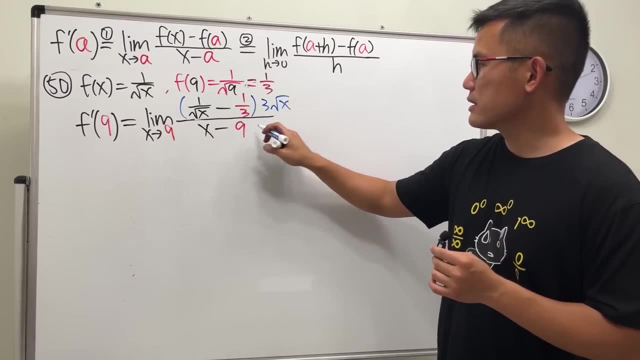 A small fraction inside of a big fraction. Second thing is we have square root. By the way, let's take care of the complex fraction first. Multiply the top and bottom by this and that, So we have square root of x. Okay, 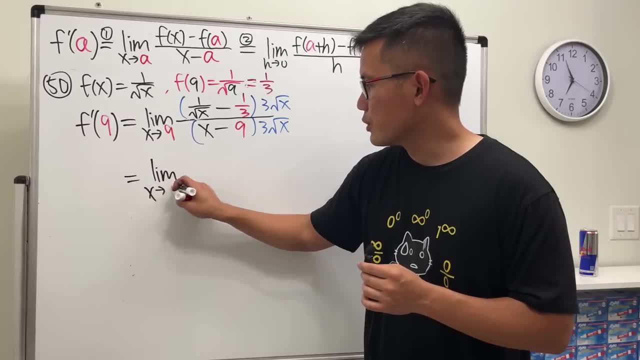 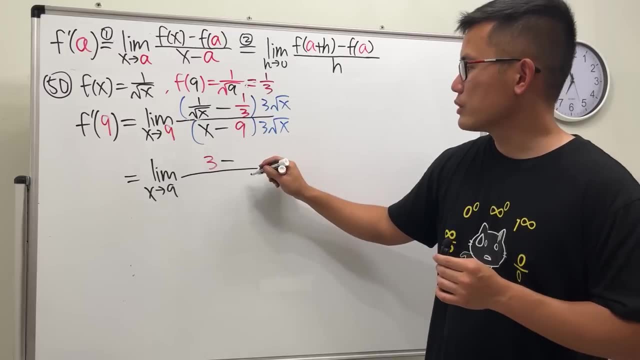 So we see this is the limit as x approaching 9.. This times that square root of x will cancel, So we have 3.. And then minus 3 cancels, So we have square root of x. I'm just going to keep them. 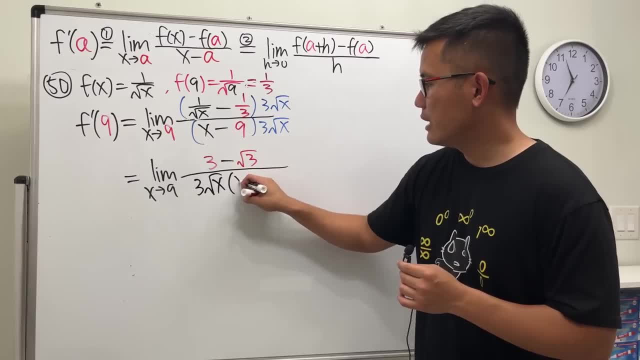 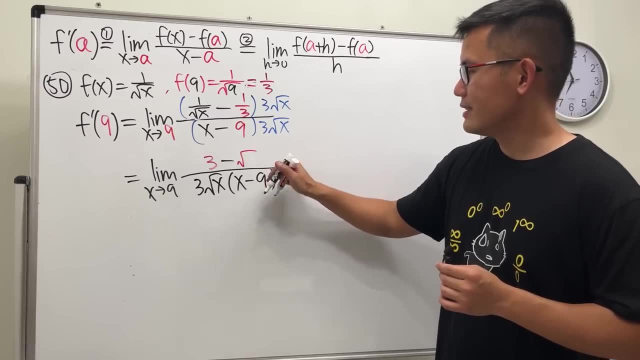 as how they are. So we have 3 square root of x times x minus 9.. Oh, hold on, hold on, hold on. This is square root of x. My bad, Alright. So for the top, I'm going to change the. 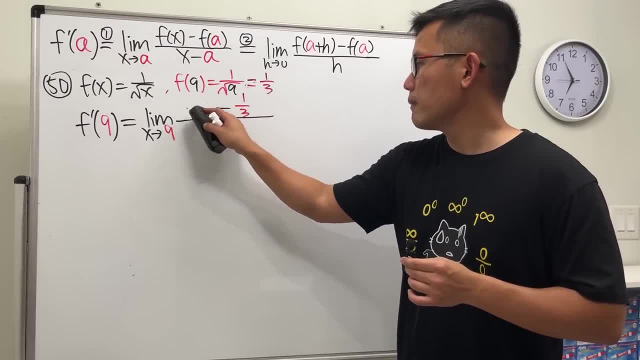 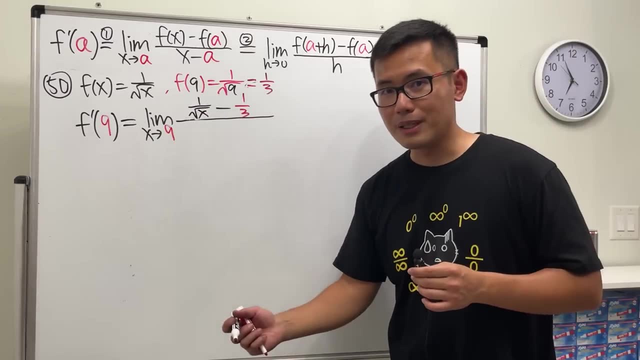 1, 3rd, 1, 3rd. let me just write it down better for you. let me just write it down better for you. let me just write it down better for you guys. what's on the bottom X minus 9, yay, guys. what's on the bottom X minus 9, yay. 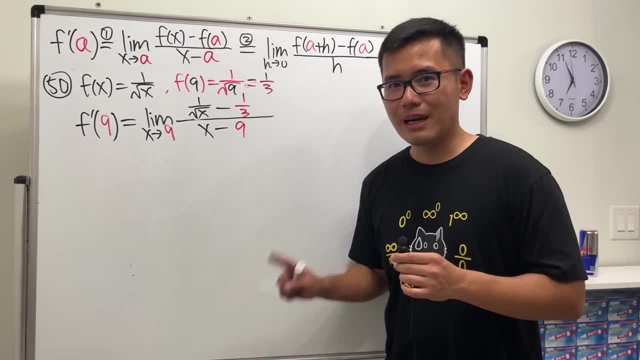 guys, what's on the bottom? X minus 9? yay, okay, here we have two things to worry. okay, here we have two things to worry. okay, here we have two things to worry. one: we have a complex fraction, a small one. we have a complex fraction, a small. 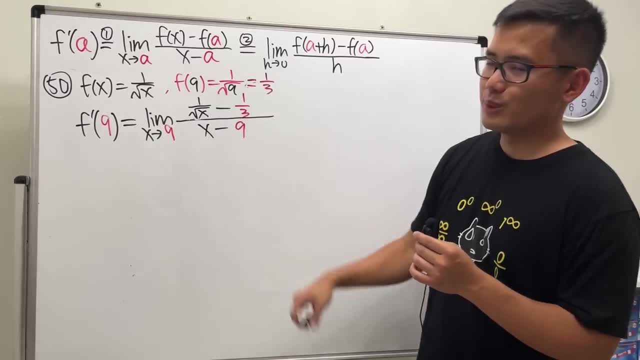 one. we have a complex fraction, a small fraction inside of a big fraction. fraction inside of a big fraction, fraction inside of a big fraction. second thing is: we have square root. yeah. second thing is we have square root- yeah. second thing is we have square root- yeah. by the way, let's take care of the. by the way, let's take care of the. by the way, let's take care of the complex fraction first. multiply the top- complex fraction first. multiply the top- complex fraction first. multiply the top and bottom by this and that, so it's 3, and bottom by this and that, so it's 3. 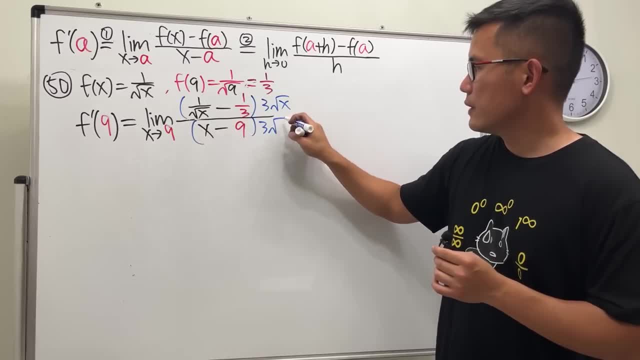 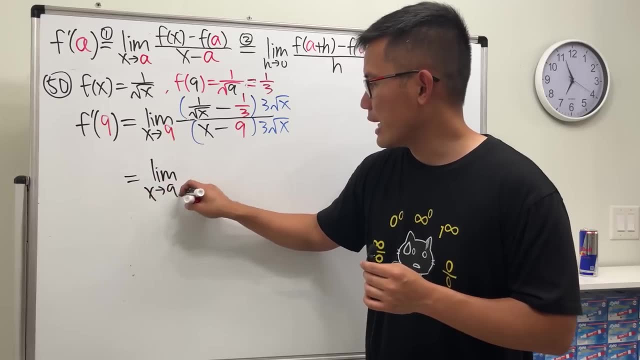 and bottom by this and that, so it's 3 square root of X. okay, so we see this is square root of X. okay, so we see this is square root of X. okay, so we see this is the limit as X approaching 9 this times. the limit as X approaching 9 this times. 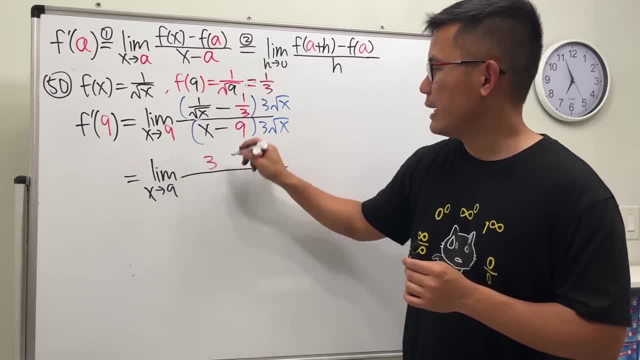 the limit as X approaching 9. this times that square root of X will cancel. so we that square root of X will cancel. so we that square root of X will cancel. so we have 3 and then minus 3- cancel. so we have 3 and then minus 3- cancel. so we. 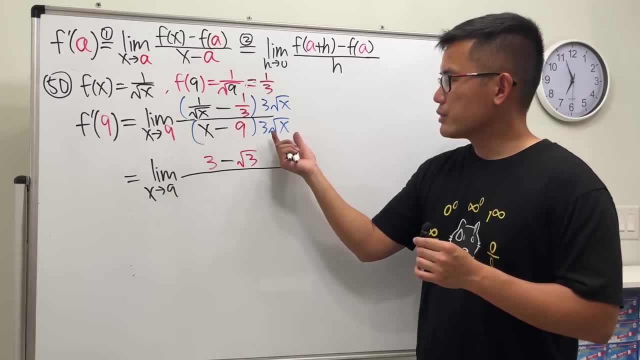 have 3 and then minus 3: cancel. so we have square root of X. I'm just going to have square root of X. I'm just going to have square root of X. I'm just going to keep them as how they are. so we have 3. 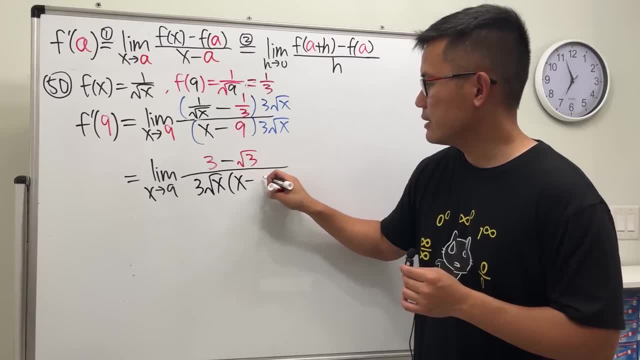 keep them as how they are, so we have 3. keep them as how they are, so we have 3. square root of X times X minus 9. square root of X times X minus 9. square root of X times X minus 9. oh, hold on, hold on. this is square root. 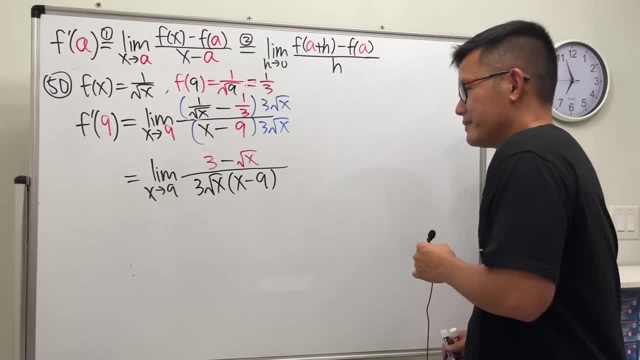 oh, hold on hold on, this is square root. oh, hold on hold on, this is square root effects. my bed all right. so for the top effects, my bed all right. so for the top effects, my bed all right. so for the top, I'm going to change the water of. 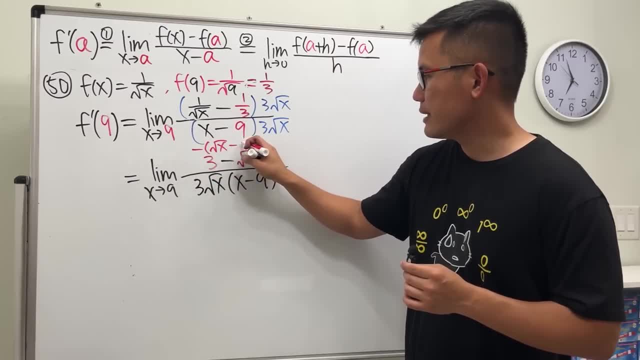 I'm going to change the water of. I'm going to change the water of subtraction. this is negative square root subtraction. this is negative square root subtraction. this is negative square root of X minus 3. I switch to water and put. of X minus 3. I switch to water and put. 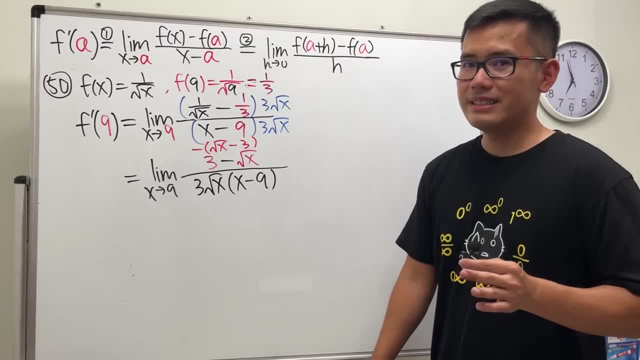 of X minus 3, I switch to water and put a negative on the outside for this. let's a negative on the outside for this. let's a negative on the outside for this. let's not do the country anymore, so just look. not do the country anymore, so just look. 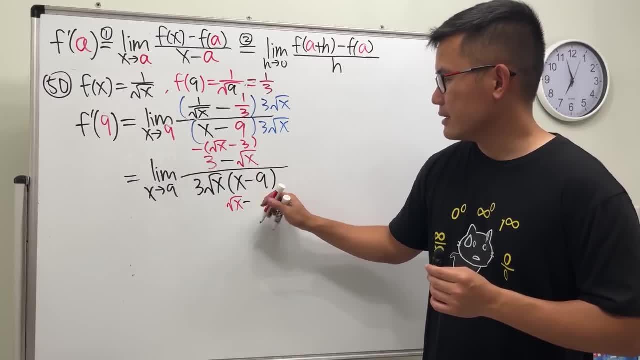 not do the country anymore. so just look at this and the factor we get square at this, and the factor we get square at this, and the factor we get: square root of X minus 3 times square root of X. root of X minus 3 times square root of X. 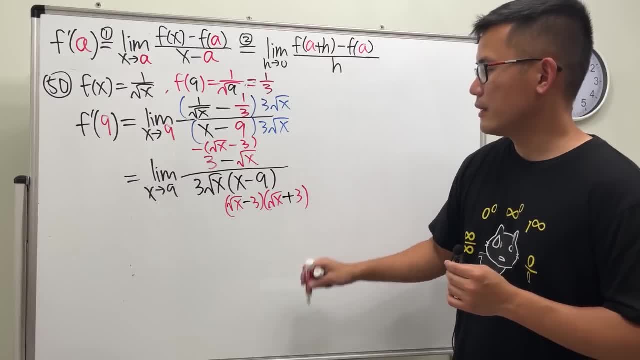 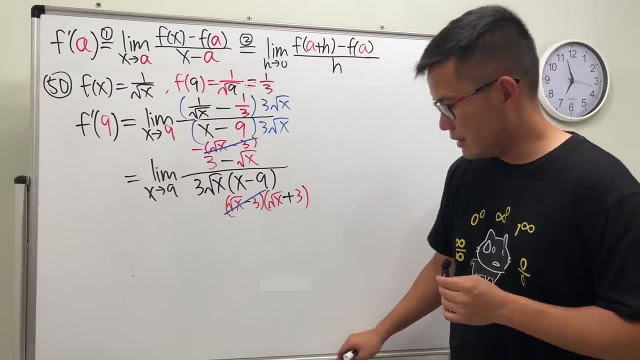 root of X minus 3 times square root of X plus 3. all right, so now you see this plus 3. all right, so now you see this plus 3. all right, so now you see this, and that can sort completely very nice, and that can sort completely very nice. 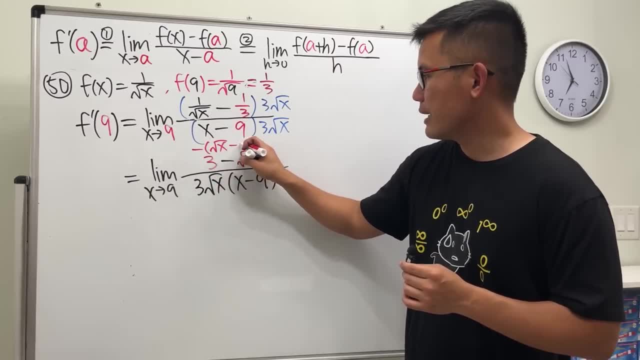 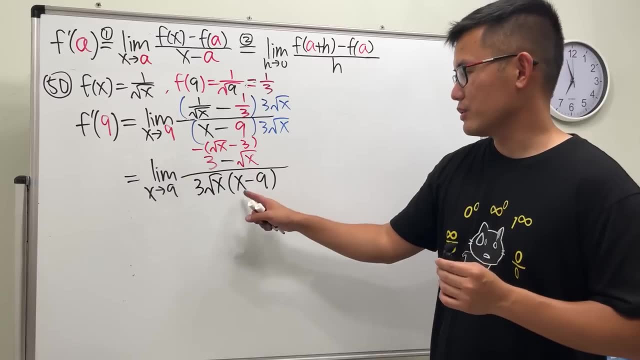 order of subtraction. This is negative square root of x minus 3.. I switch the order and put a negative on the outside For this. let's not do the counting anymore. So just look at this: in a factor We get square root of x. 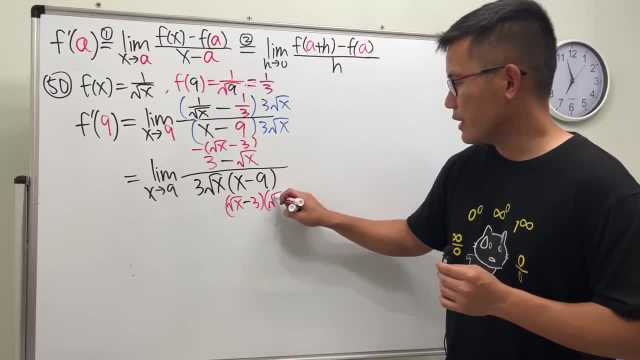 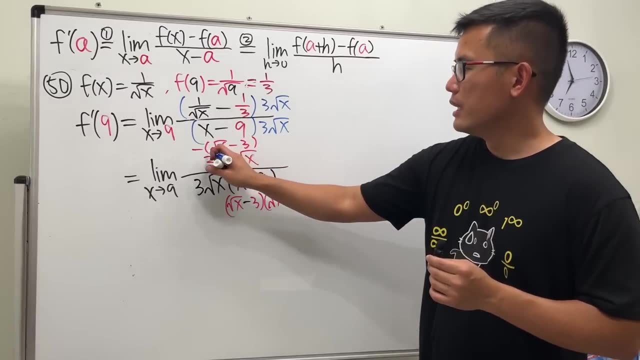 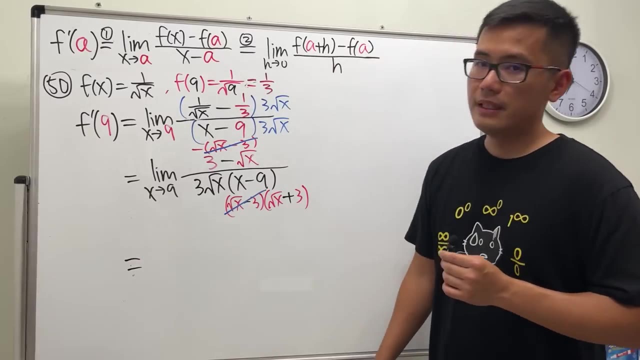 minus 3 times square root of x plus 3.. Alright, So now you see this and that cancel out completely. Very nice. So, ladies and gentlemen, on the top we have negative 1, over here we have 3, and then here we have. 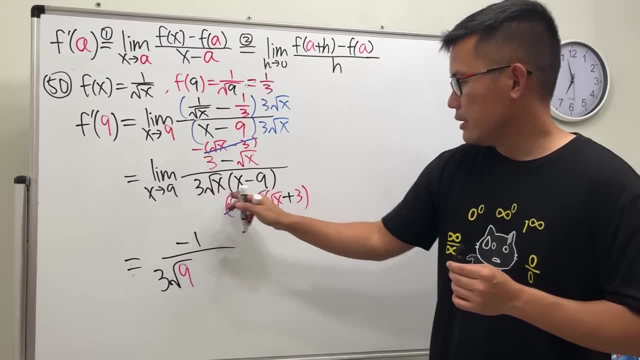 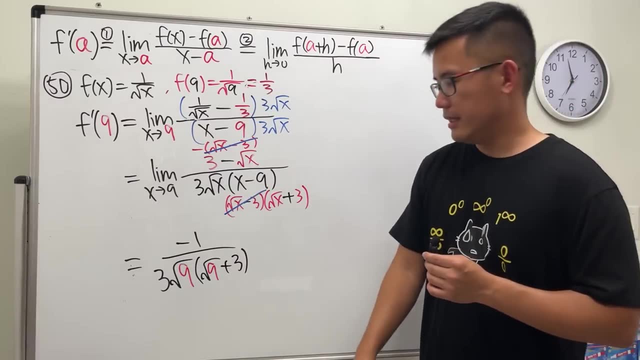 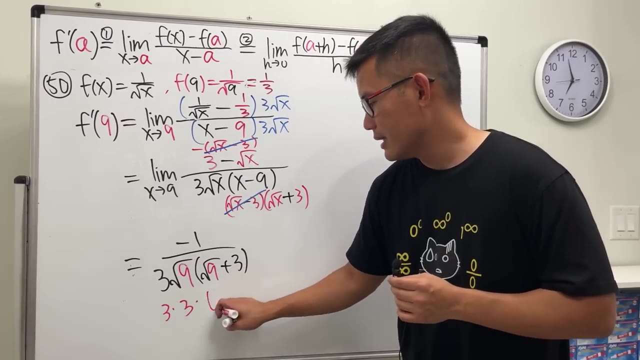 square root of x, x is 9.. That's gone. And then here we have square root of 9 plus 3.. Yeah, And now we just have to work this out. This is 3 times 3 times 3 plus 3 is 6.. 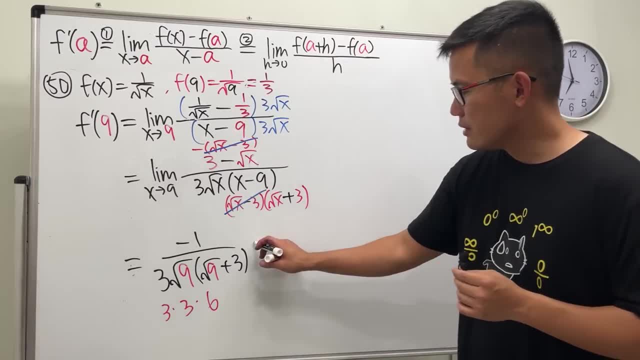 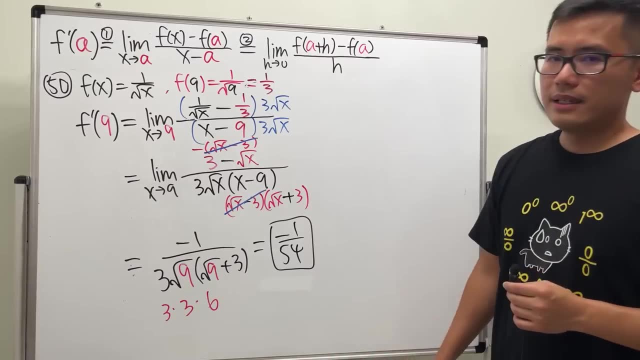 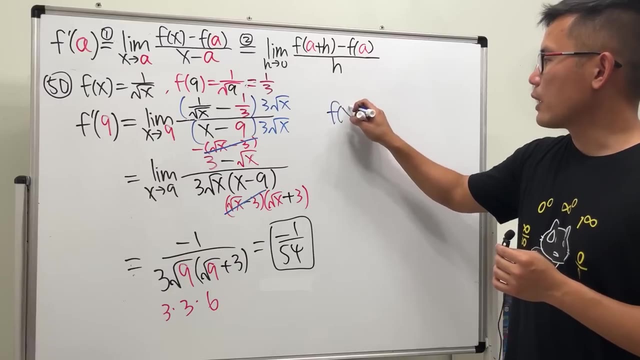 9 times 6 is 54. So all together, we get negative 1 over 54.. Done, Give you guys a small bonus right here. In fact, we can also use the power rule for this question. Check this out When we have our function. 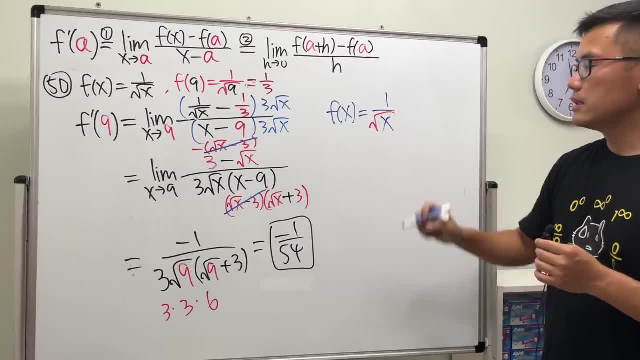 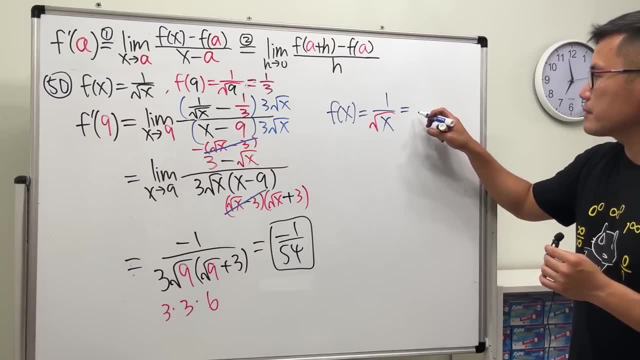 this is 1 over square root of x. In calculus a lot of times we look at the square root as the 1 half power. So this right here is the same as saying x to the 1 half power. But we can bring that up. So this right here is actually: 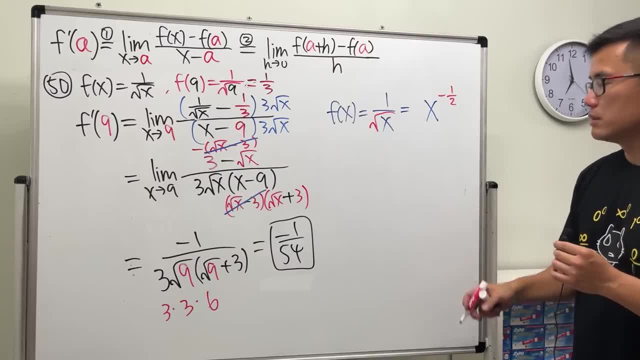 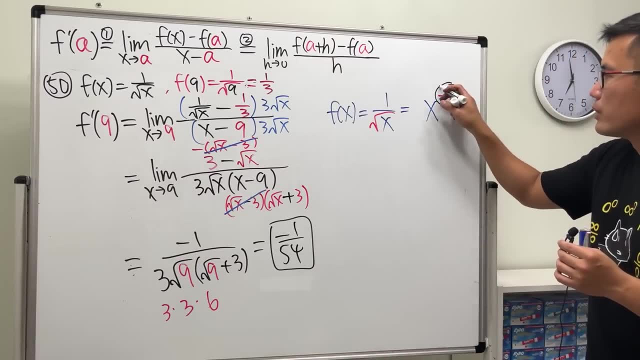 just x to the negative 1 half power. Okay, And the reason that we want to do this is because we can use the power rule. Check this out: Put the power to the front and then minus 1. So we get f prime. 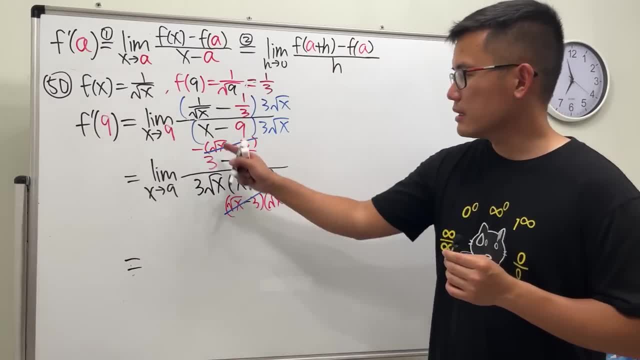 and that can sort completely very nice. so, ladies and gentlemen on the top, we so, ladies and gentlemen on the top. we so, ladies and gentlemen on the top, we have negative 1 over here, we have 3. and have negative 1 over here, we have 3, and 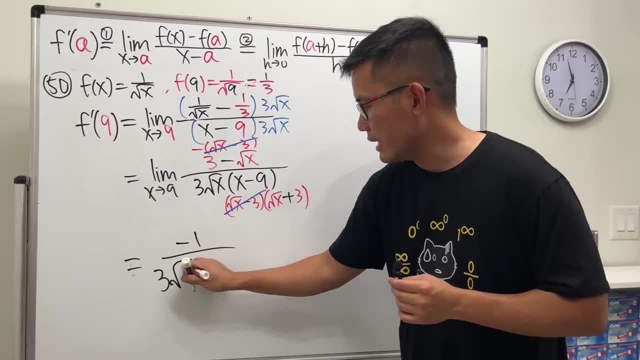 have negative 1 over, here we have 3, and then here we have square roots of X- X. then here we have square roots of X- X. then here we have square roots of X- X is 9, that's gone. and then here we have is 9, that's gone. and then here we have. 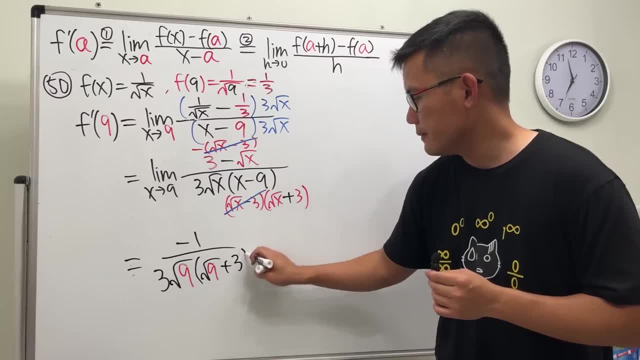 is 9. that's gone. and then here we have square root of 9 plus 3- yeah, and now square root of 9 plus 3- yeah, and now square root of 9 plus 3- yeah, and now, just how to work this out, this is 3. 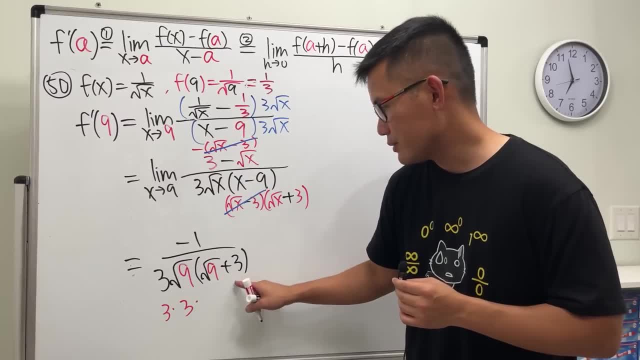 just how to work this out. this is 3. just how to work this out. this is 3 times 3 times 3 plus 3 is 6, 9 times 6, is times 3 times 3 plus 3 is 6, 9 times 6 is. 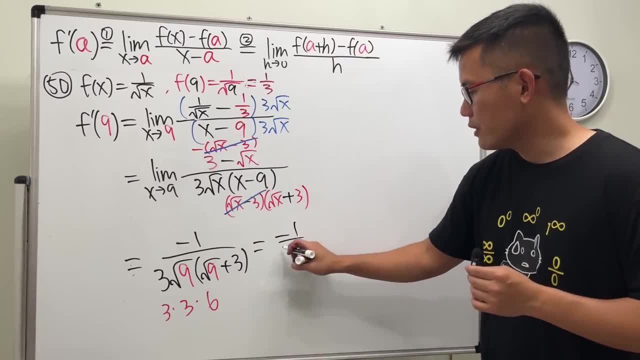 times 3 times 3 plus 3 is 6. 9 times 6 is 54. so all together we get negative 1- 54. so all together we get negative 1- 54. so all together we get negative 1 over 54 done, if you get a small bonus. 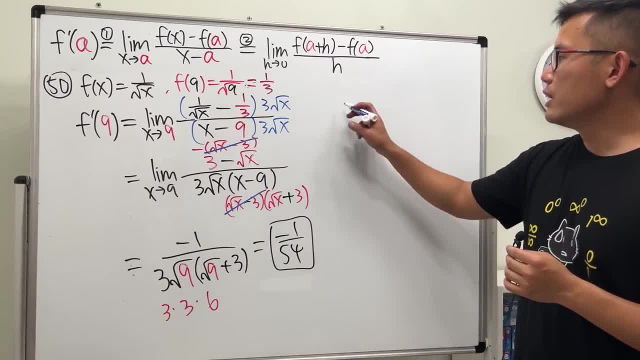 over 54 done. if you get a small bonus over 54. done. if you get a small bonus right here. in fact, we can also use the right here. in fact, we can also use the right here. in fact, we can also use the power rule for this question. check this. 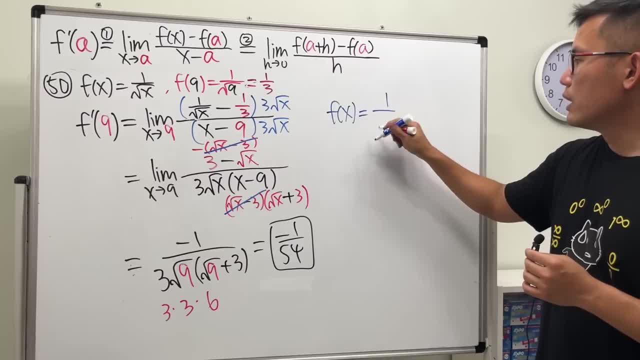 power rule for this question. check this power rule for this question. check this out when we have our function. this is 1 out when we have our function. this is 1 out when we have our function. this is 1 over square root of X in calculus. a lot. 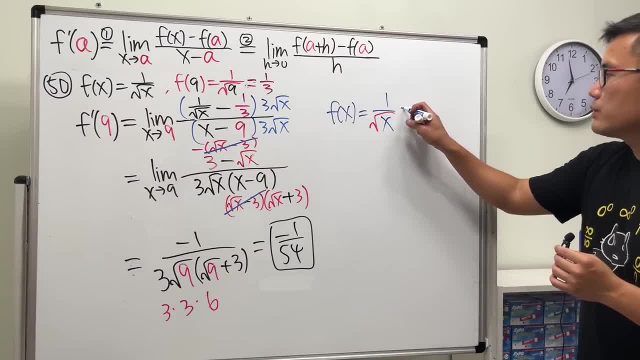 over square root of X in calculus, a lot over square root of X in calculus. a lot of times we look at the square root. as of times we look at the square root as of times we look at the square root as the 1 half power. so this, right here it's. 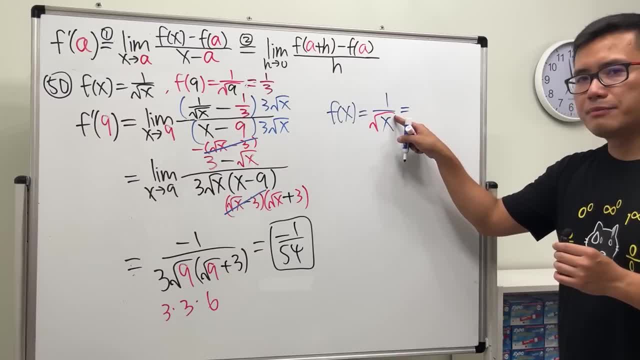 the 1 half power. so this right here, it's the 1 half power. so this right here, it's the same as saying X to 1 half power, the same as saying X to 1 half power, the same as saying X to 1 half power, but we can bring that up. so this right. 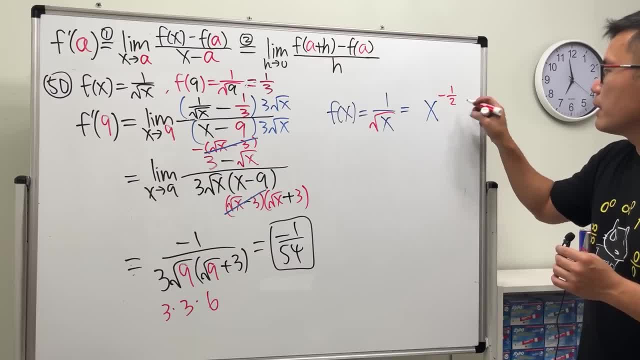 but we can bring that up, so this right, but we can bring that up, so this right. here it's actually just X to the here. it's actually just X to the here. it's actually just X to the negative 1 half power: okay, and the negative 1 half power: okay, and the. 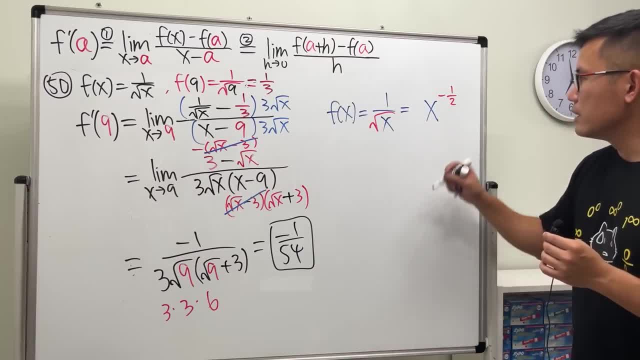 negative 1 half power. okay, and the reason that we want to do this is reason that we want to do this is reason that we want to do this is because we can use the power rule check, because we can use the power rule check, because we can use the power rule check this out, put the power to the front and 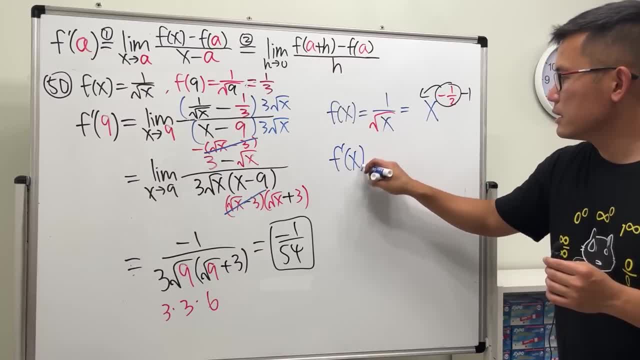 this out: put the power to the front and this out: put the power to the front and then minus 1, so we get f prime of X and then minus 1, so we get f prime of X and then minus 1, so we get f prime of X and we get negative 1 over 2 at the front. 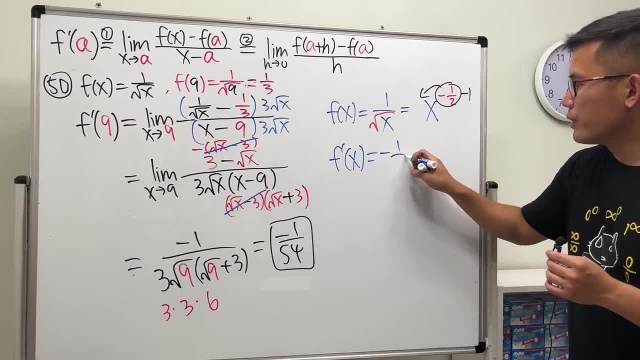 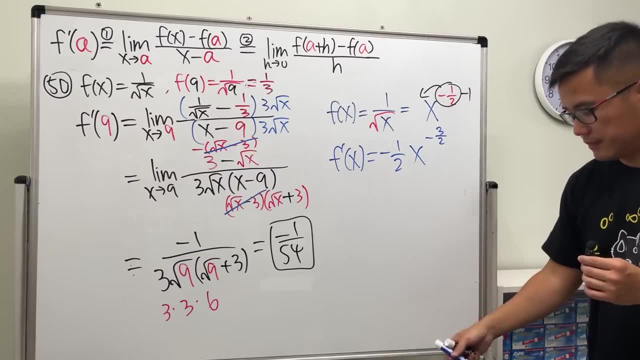 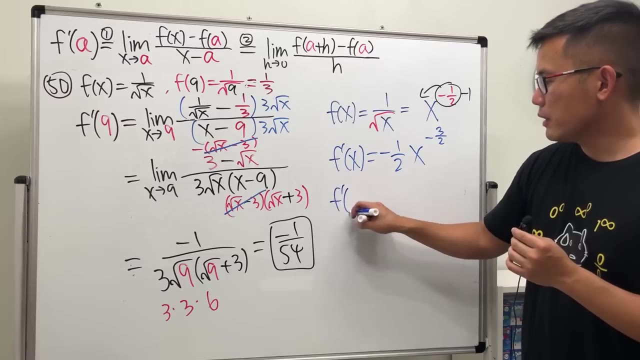 of x And we get negative 1 over 2 at the front And x, This minus that is negative 3 over 2.. Yeah, What's next? Well, we want f prime of 9.. Yeah, So f prime of 9.. 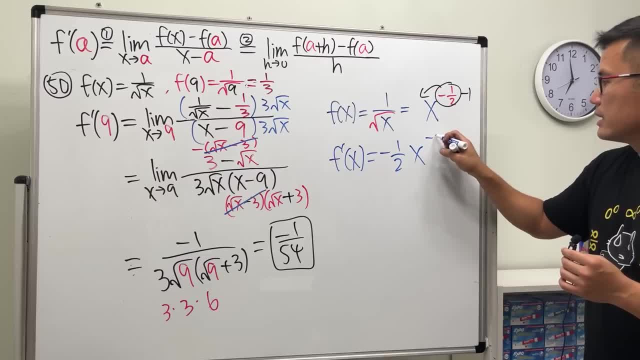 we get negative 1 over 2 at the front. we get negative 1 over 2 at the front, and then X- this minus dies negatives 3, and then X- this minus dies negatives 3, and then X- this minus dies negatives- 3 over 2. yeah, what's next? well, we want f. 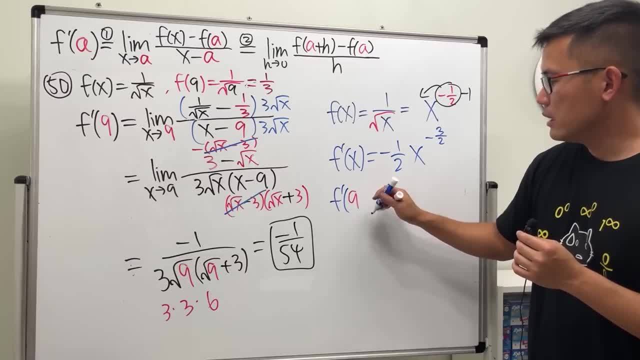 over 2. yeah, what's next? well, we want f over 2. yeah, what's next? well, we want f prime of 9. yeah, so f prime of 9, this prime of 9. yeah, so f prime of 9, this prime of 9. yeah, so f prime of 9. this right here gives us negative. let me just 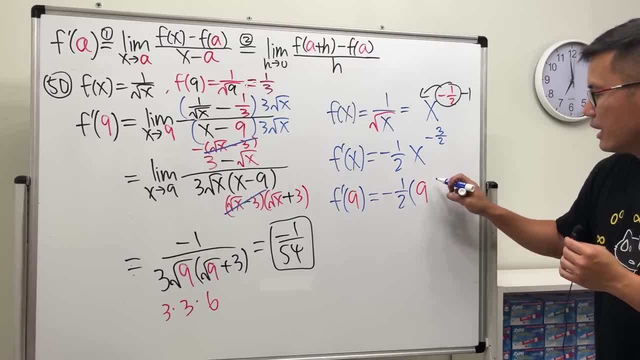 right here gives us negative. let me just right here: gives us negative. let me just write it down: negative 1 half, and then write it down negative 1 half, and then write it down negative 1 half, and then we have 9, and then to the negative 3. 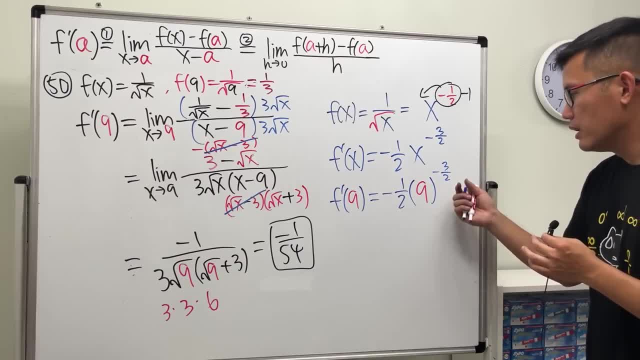 we have 9, and then to the negative 3. we have 9, and then to the negative 3: half power. the main question is: how do we half power? the main question is: how do we half power? the main question is: how do we simplify this? if we can do it, then 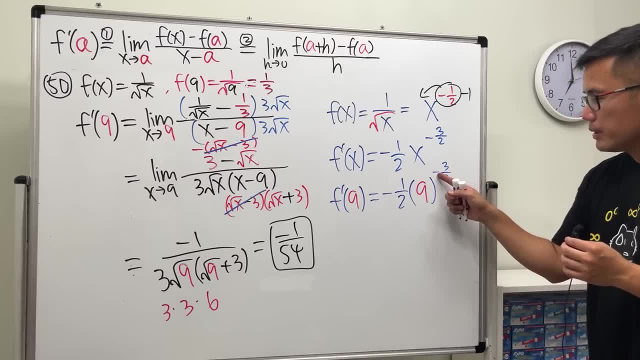 simplify this. if we can do it, then simplify this. if we can do it, then we're done. yeah, so usual thing, put the we're done. yeah, so usual thing, put the we're done. yeah, so usual thing, put the power right if it's a negative power. 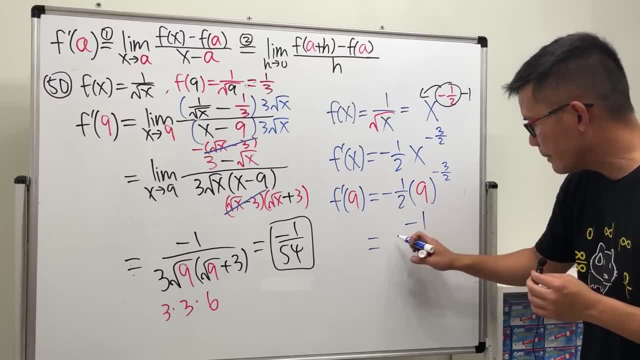 power right. if it's a negative power, power right. if it's a negative power, then put it to the bottom. so this right, then put it to the bottom. so this right, then put it to the bottom. so this right here is negative. 1 on the top over 2. 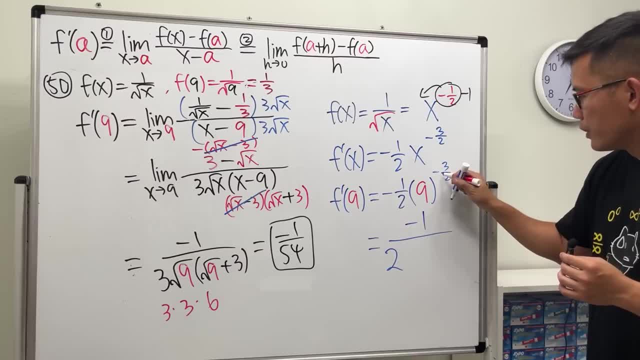 here is negative 1 on the top over 2. here is negative 1 on the top over 2, and then, and then, and then, once we bring this down to the bottom, once we bring this down to the bottom, once we bring this down to the bottom, we have the over 2 right here. right, let's. 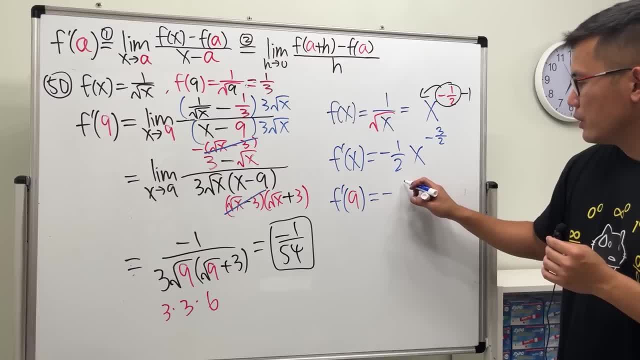 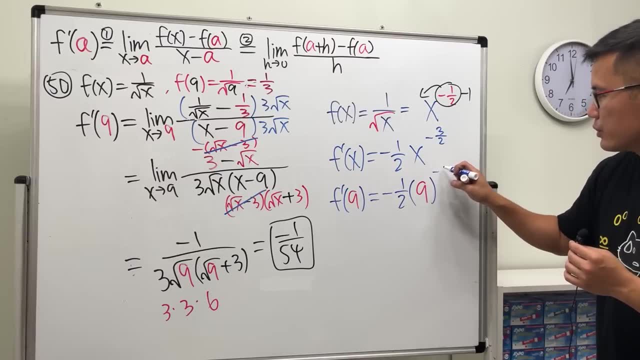 This right here gives us negative- Yeah, Let me just write it down: Negative 1 half, and then we have 9, and then to the negative 3 half power. The main question is: how do we simplify this? if we can do it, Then we are done, Yeah, So 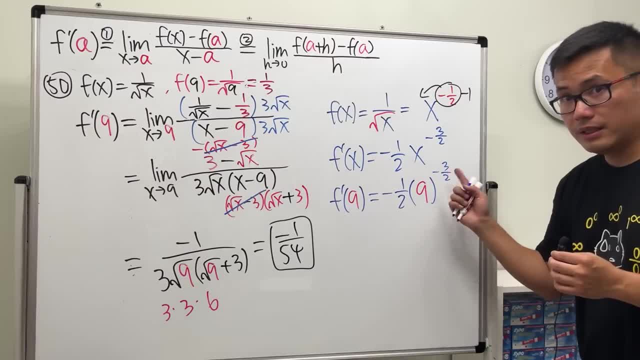 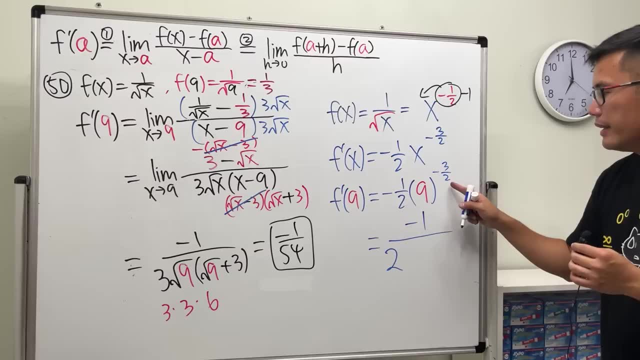 usual thing: Put the power right. If it's a negative power, then put it to the bottom. So this right here is negative 1 on the top over 2.. And then, once we bring this down to the bottom, we have the over 2. 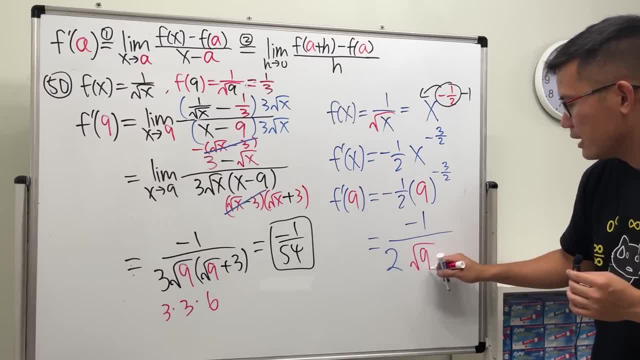 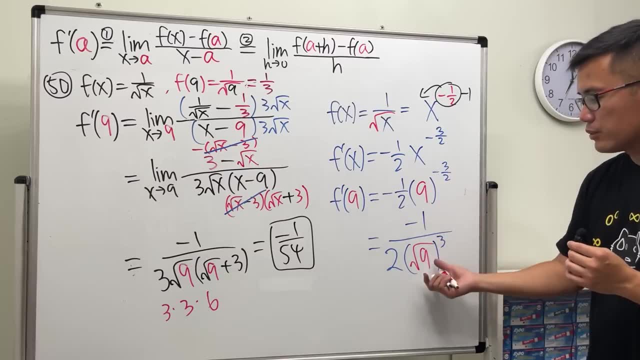 right here? right, Let's change that to a square root, And then we have the 9. And then raise that to the third power. So that's pretty much how we do it. Okay, This negative. bring this down to the bottom. 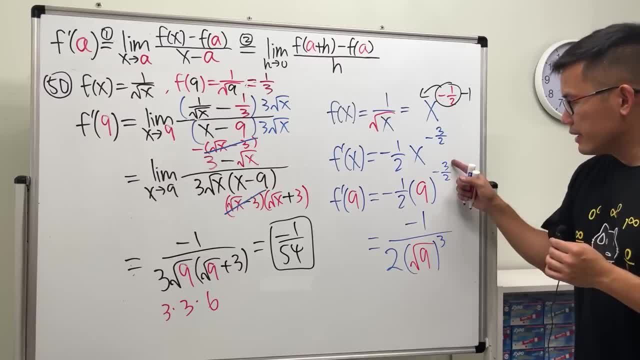 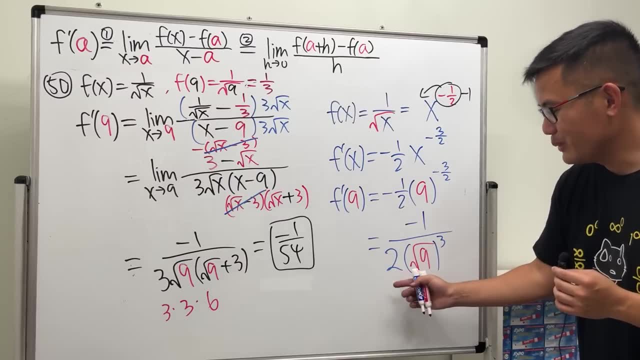 The over 2 power change to the square root And then the third power stays And you see, square root of 9 is 3.. 3 to the third power is 27.. Times 2 is 54.. And that's on the bottom. 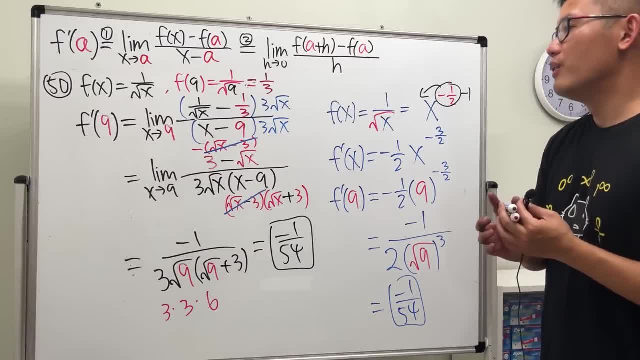 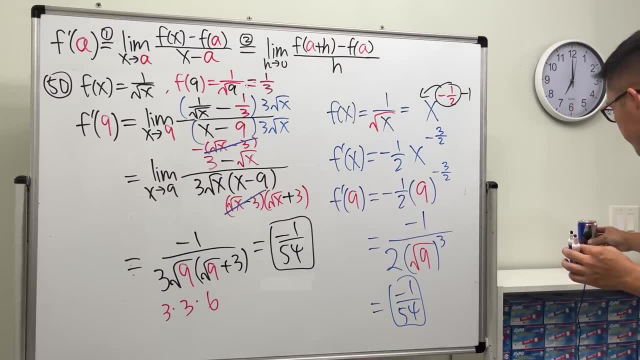 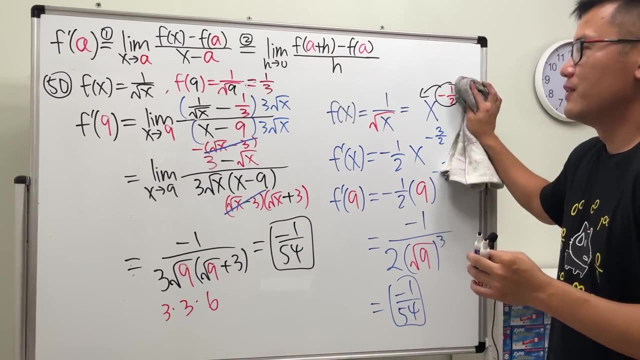 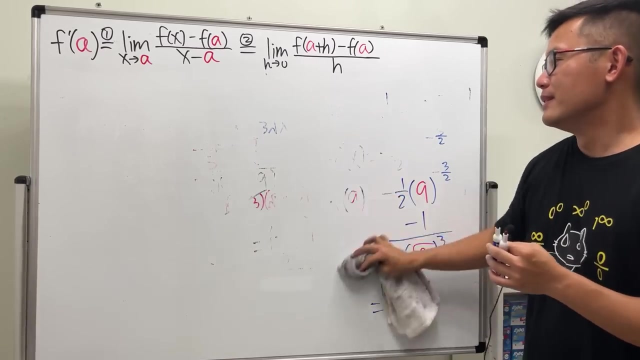 All in all, negative 1 over 54.. How cool is that, huh? Yes, No, I'm not done yet, I know, but I still have like 50 more to go, 51 more to go. Actually, I don't know. 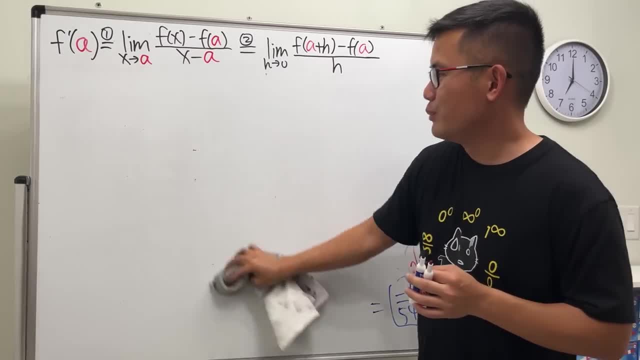 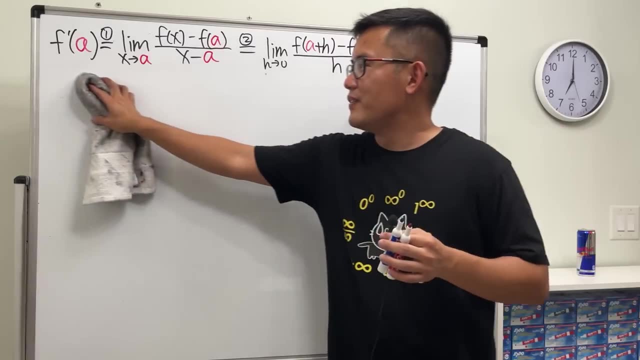 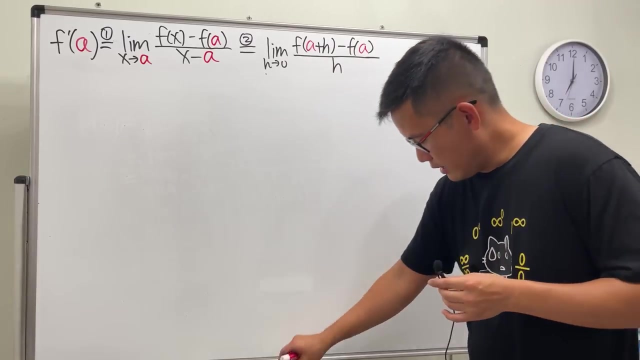 if it's 50 or 51. I'm not really Go see, Go see, All right. So I think that's it for this video. Thank you for watching. See you next time. Bye, Bye, Next, we want to. 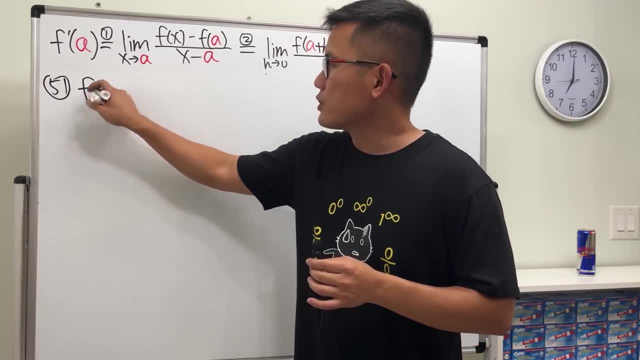 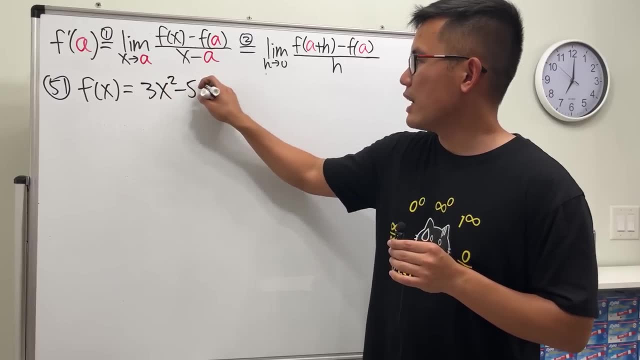 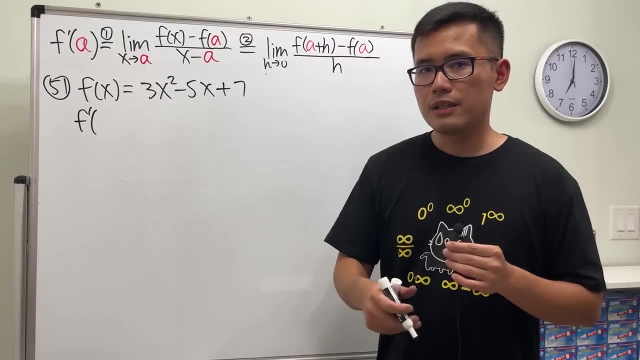 do this 51.. We are given the function f of x, And this is just a regular polynomial, It's quadratic. We have 3x squared minus 5x plus 7.. Instead of saying f prime of like 2, f prime of. 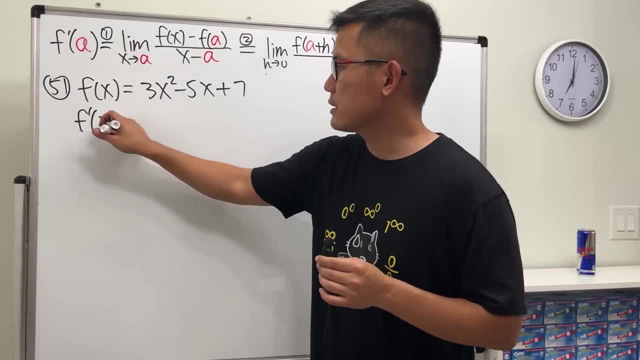 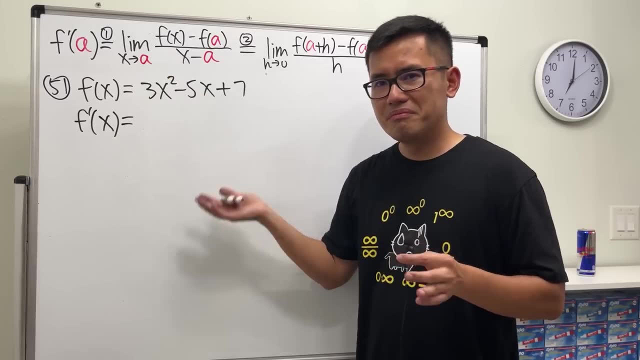 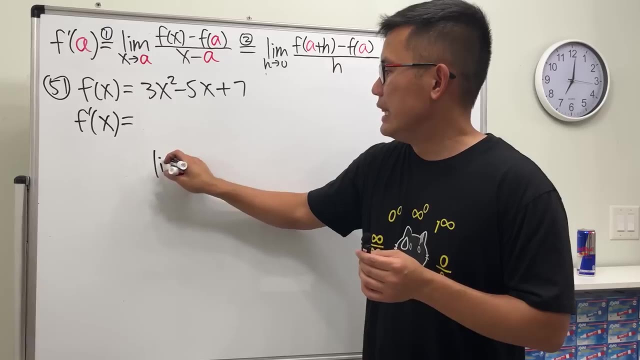 negative 7, we want f prime of just x. So now here's the trouble. We still use definition 1.. Kind of, If you put this x, If you make this x red, then you are talking about the limit as this x approaching. 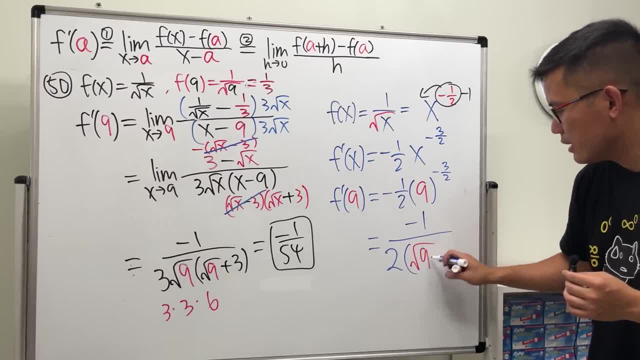 we have the over 2 right here. right, let's. we have the over 2 right here. right, let's change that to a square root, and then we change that to a square root, and then we change that to a square root, and then we have the 9, and then. 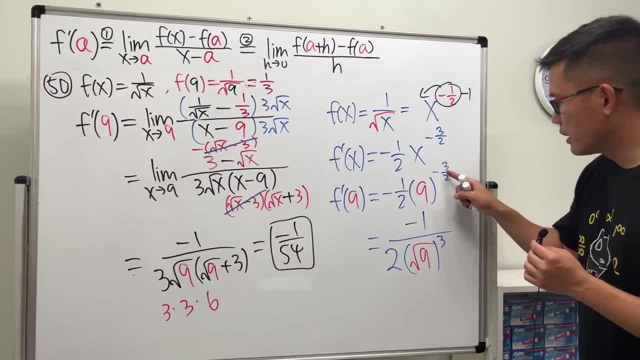 have the 9 and then have the 9 and then raise that to the third power. so that's raise that to the third power. so that's raise that to the third power. so that's pretty much how you do it again this, pretty much how you do it again this. 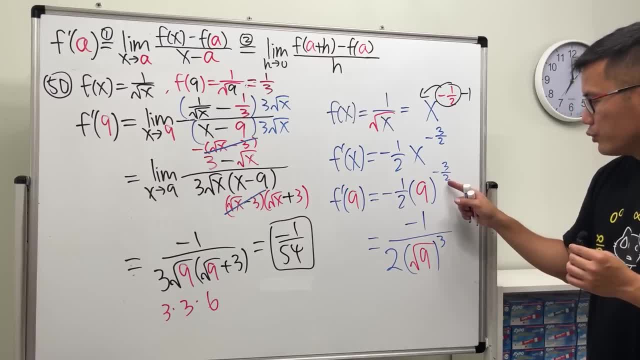 pretty much how you do it again. this negative- bring this down to the bottom. negative, bring this down to the bottom. negative, bring this down to the bottom. the over 2 power change to the square. the over 2 power change to the square. the over 2 power change to the square root. 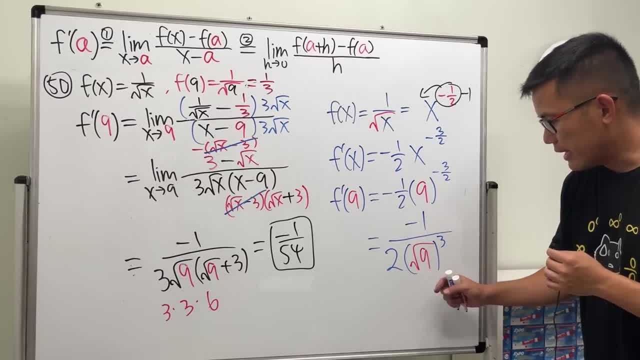 root root, and then the third power stays, and you, and then the third power stays, and you, and then the third power stays, and you see, see, see, square root of 9 is 3: 3 to the third. square root of 9 is 3: 3 to the third. 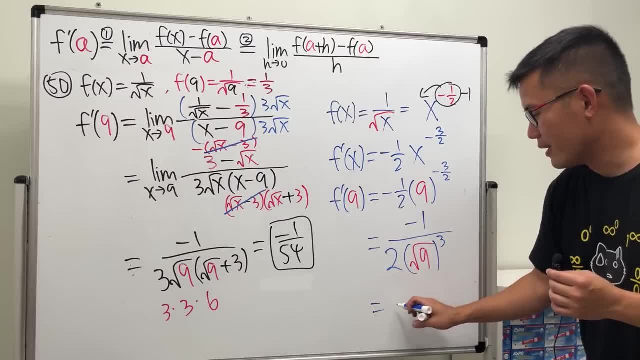 square root of 9 is 3. 3 to the third: power is 27, power is 27, power is 27 times 2 is 54 times 2 is 54 times 2 is 54. and that's on the bottom and that's on the bottom. 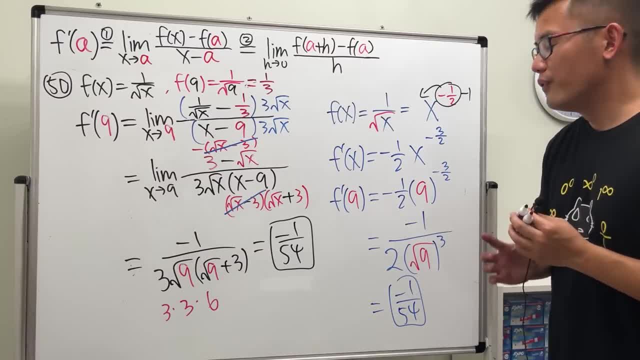 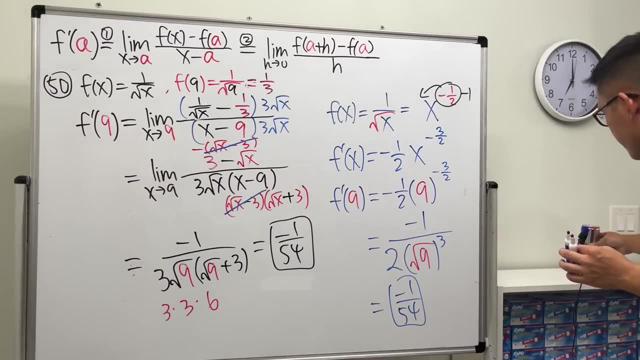 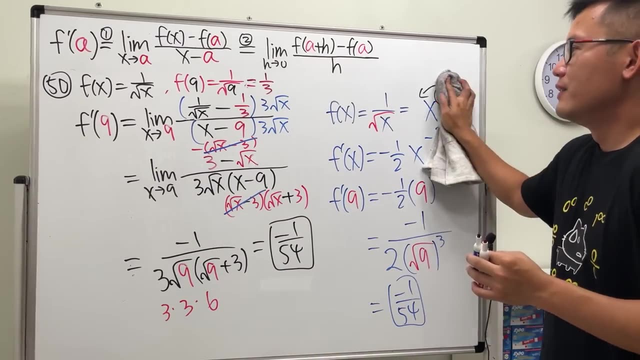 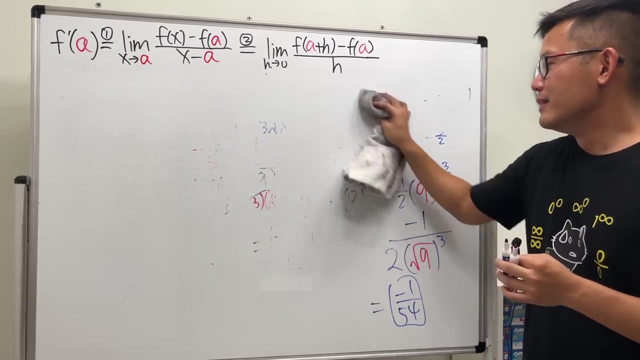 and that's on the bottom. all in all: negative: 1 over 54. all in all: negative: 1 over 54. all in all: negative 1 over 54. how cool is that? yes, no, i'm not done yet, i know, but like it's not funny. yeah, i still have like. 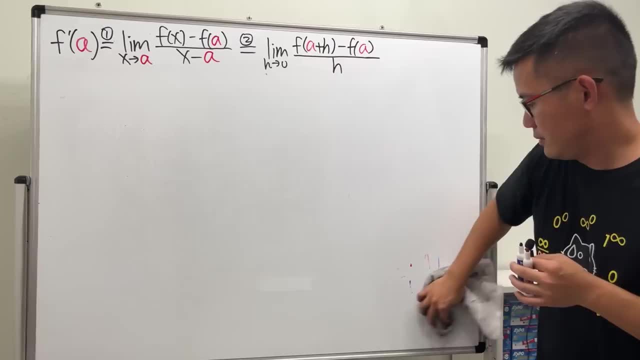 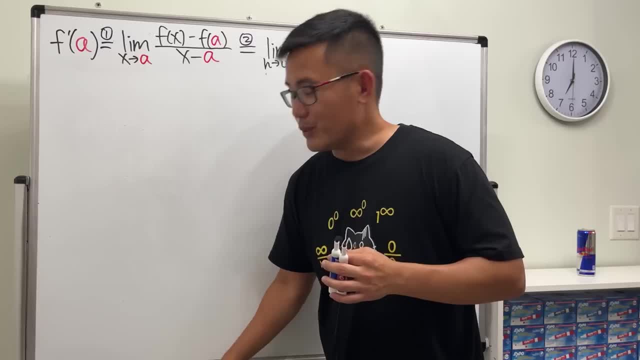 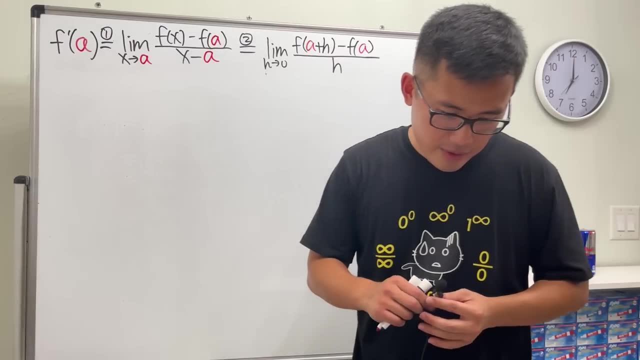 actually i don't know if it's 50 or 51. actually i don't know if it's 50 or 51, i'm not really go see, you'll see. all right next, we want to do this. all right. next, we want to do this. 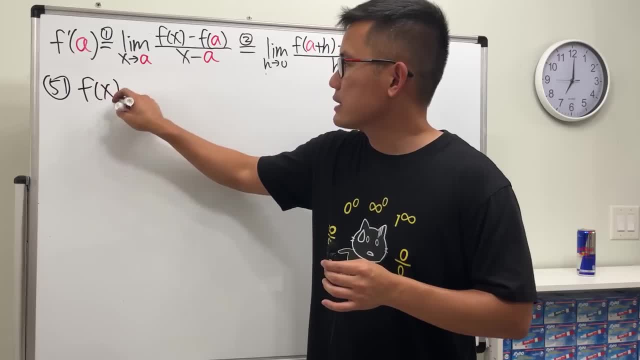 all right. next we want to do this: 51 we have given the function f of x. 51 we have given the function f of x. 51 we have given the function f of x. and this is just a regular polynomial, and this is just a regular polynomial. 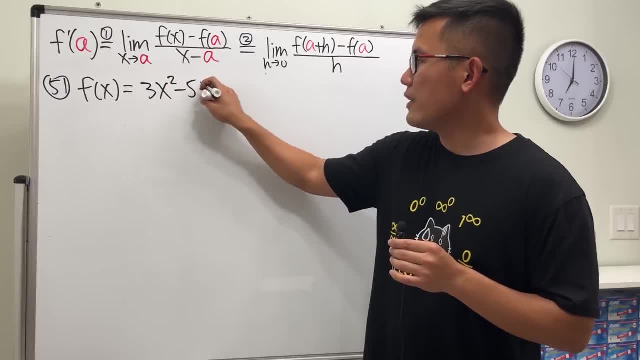 and this is just a regular polynomial. it's quadratic, it's quadratic, it's quadratic. we have 3x squared minus. we have 3x squared minus. we have 3x squared minus 5x plus 7, 5x plus 7, 5x plus 7. instead of saying f prime of like 2 f. 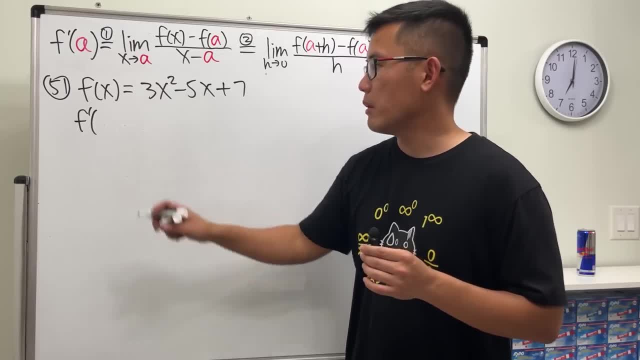 instead of saying f prime of like 2 f, instead of saying f prime of like 2, f prime of negative 7 prime of negative 7 prime of negative 7. we want f prime of just x. we want f prime of just x. we want f prime of just x. so now, here's the trouble. can we still? 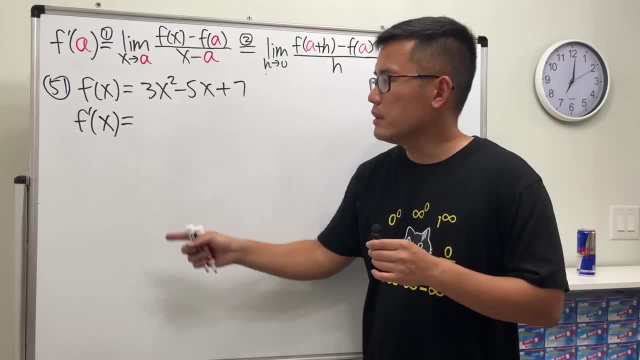 so now, here's the trouble, can we still? so now here's the trouble. can we still use definition? one use definition, one use definition, one kind of: if you put this x, kind of, if you put this x, kind of, if you put this x, if you make this x red, then you are. 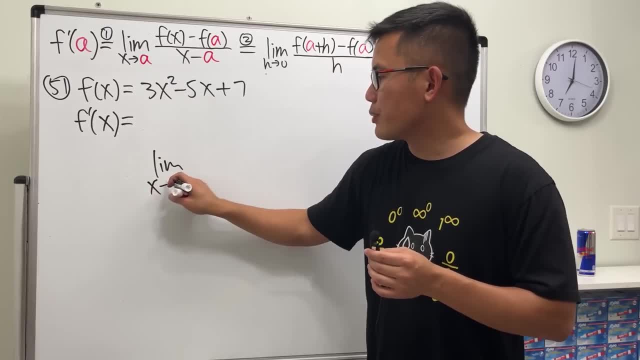 if you make this x red, then you are. if you make this x red, then you are talking about the limit, as this x. talking about the limit, as this x. talking about the limit, as this x approaching this x. right, this x is. let's approaching this x. right, this x is let's. 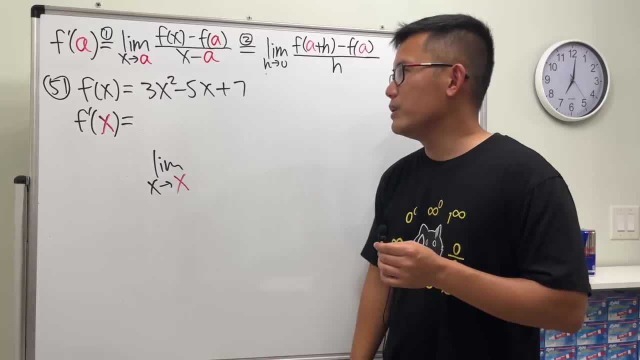 approaching this x. right, this x is: let's say it's red, say it's red, say it's red. then we can just replace that a with the, then we can just replace that a with the. then we can just replace that a with the red x, red x. 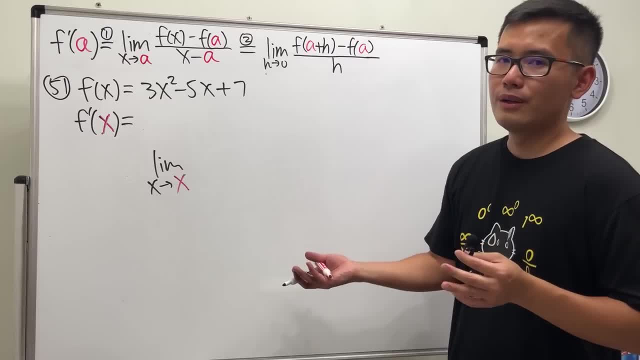 red x. but you know the deal: this does not. but you know the deal: this does not. but you know the deal, this does not. it doesn't look good at all. it doesn't look good at all. it doesn't look good at all. right, it does not look good at all, so no, 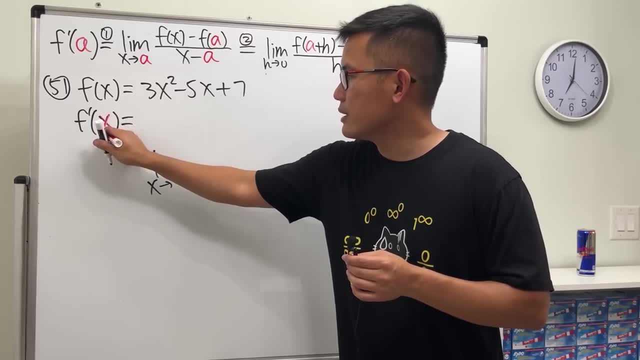 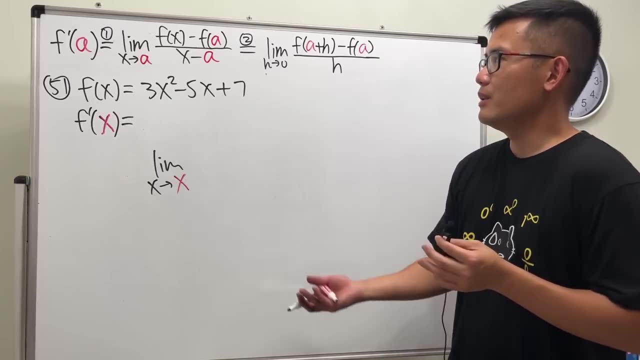 this x. This x is, let's say it's red, Then we can just replace the a with the red x. But you know the deal. This doesn't look good at all. Right, It does not look good at all. 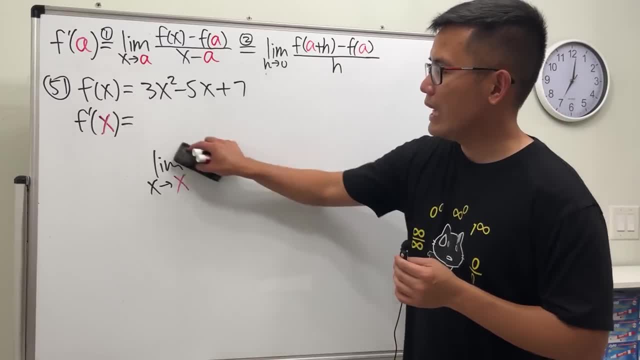 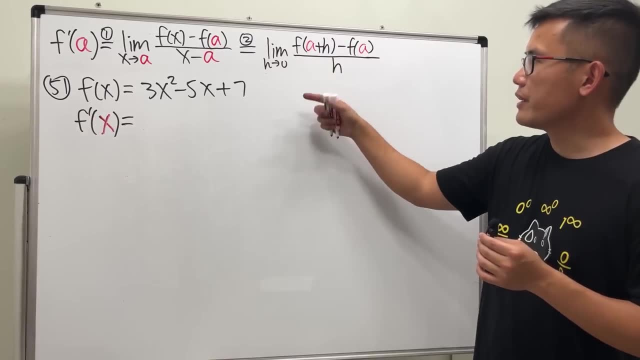 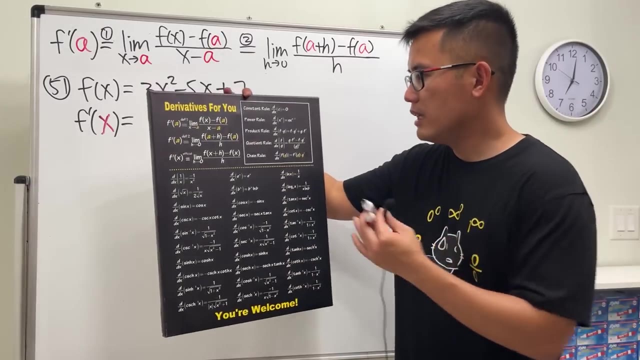 So no, That's why we have the definition 2.. If we want to do f prime of x, then we look at this right here and just replace the a with x, And it's still a jet. Yeah, see, It's the official definition of the. 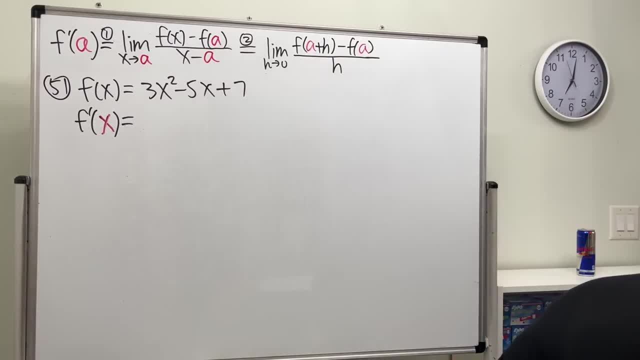 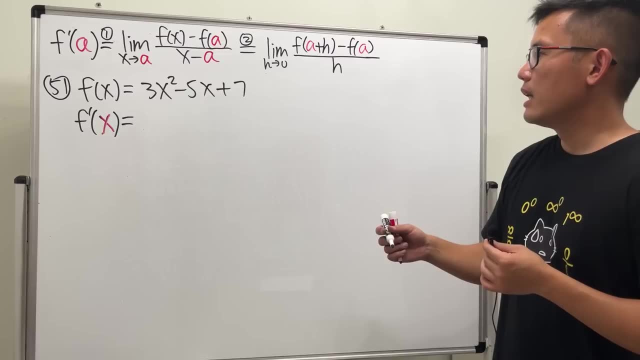 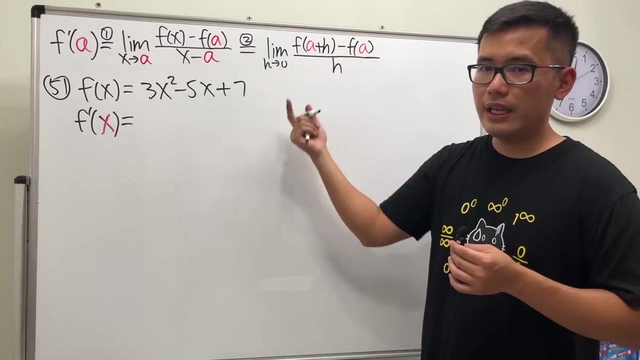 derivative. Okay, So I'm just going to- hmmm, No, I'm just going to write this right here. Here we go. We're looking at definition 2 and just change the a to x. That's all you have to remember. 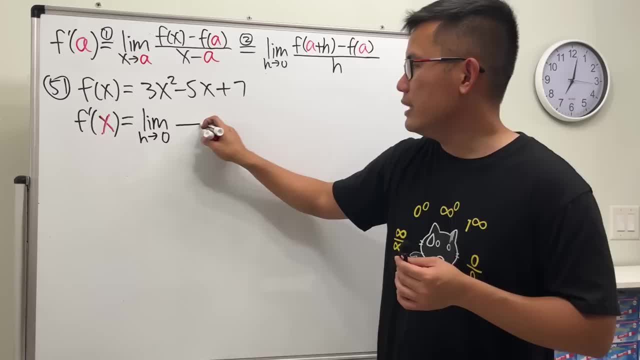 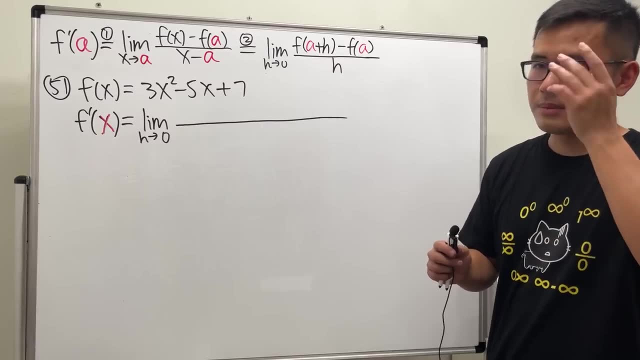 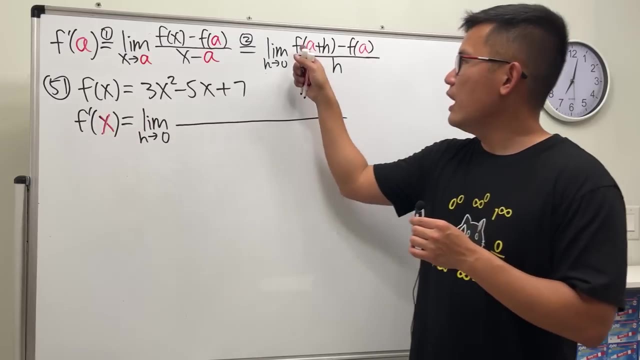 So here we have the limit as h approaching 0. And this right here, it's not easy. This is perhaps one of the first things that people dislike about the calculus part. It's pretty demanding, I would say. Anyway, we want to have f of. 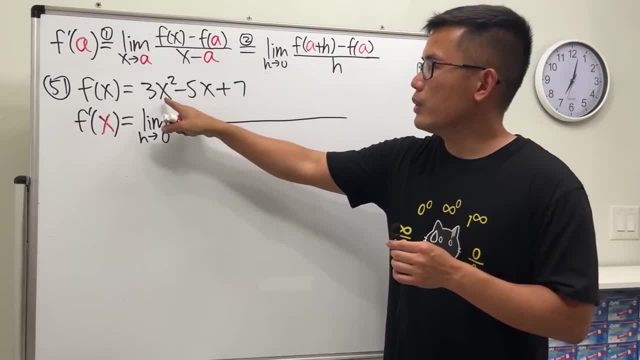 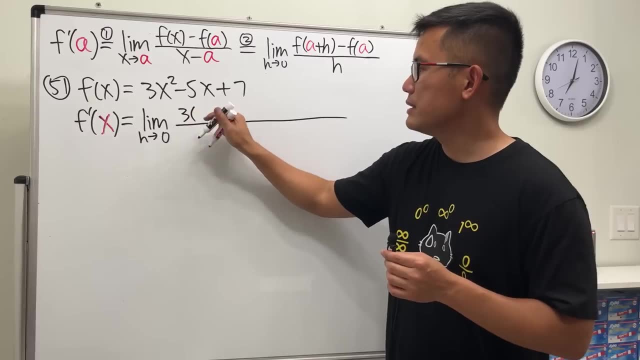 x plus h. So what that means is we want to look at all the x's here and then plug in x plus h. I'll show you. We will first get 3 times x plus h And then square that, And then you continue. 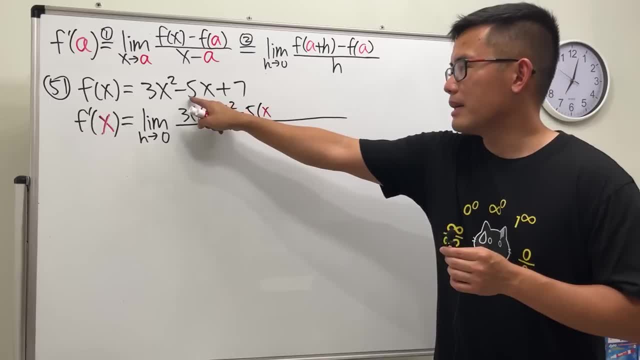 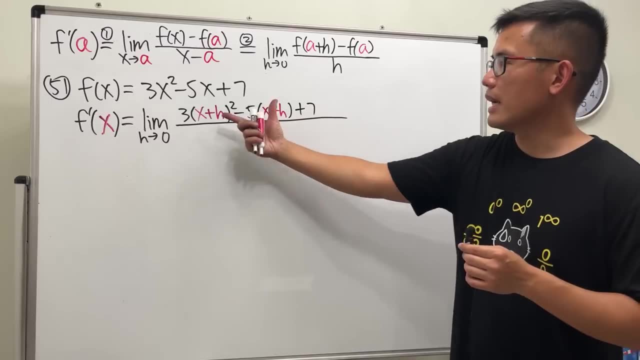 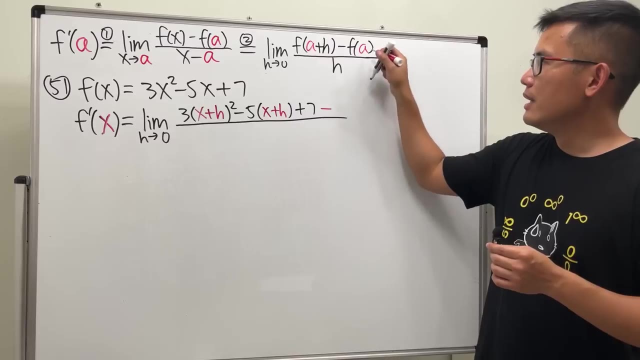 minus f of x. So minus 5 of minus 5 times x plus h And then plus 7.. So that's the f of x plus h part. And then we want to minus f of x, which is just the original. So it's. 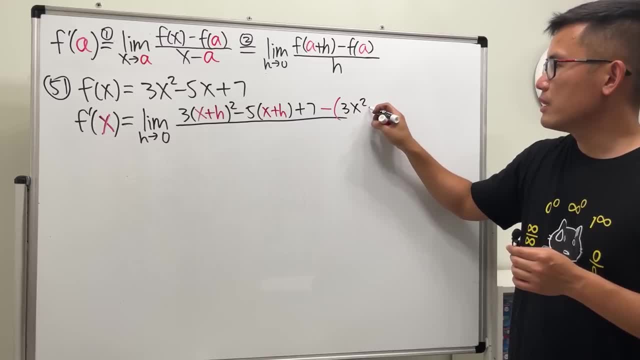 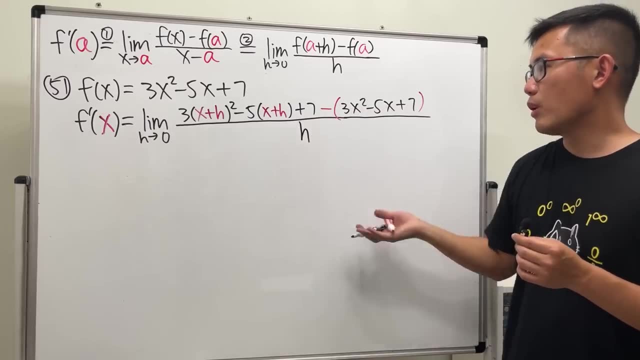 just minus. And then we just put this down: 3x squared minus 5x plus 7. And you can see that this expression is pretty long already, And perhaps it's the longest, Especially if you just come from pre-calc. 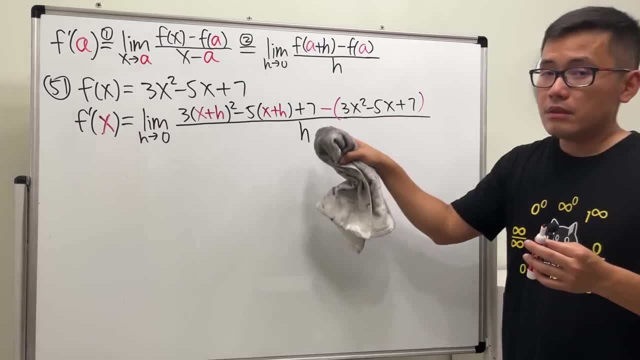 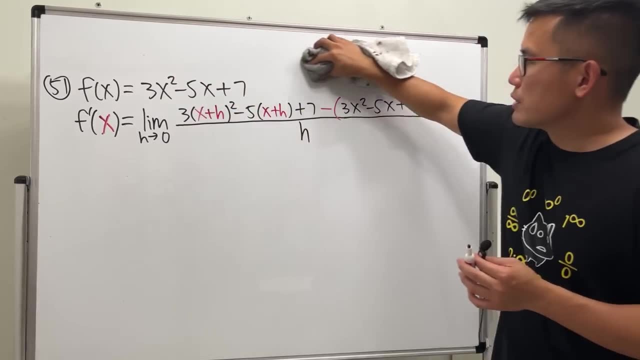 and, yeah, pretty intimidating. So that's the idea, But for now I'm just going to erase both of this, So that way we can actually just put down the definition of derivative For f, prime of x, And then we'll focus. 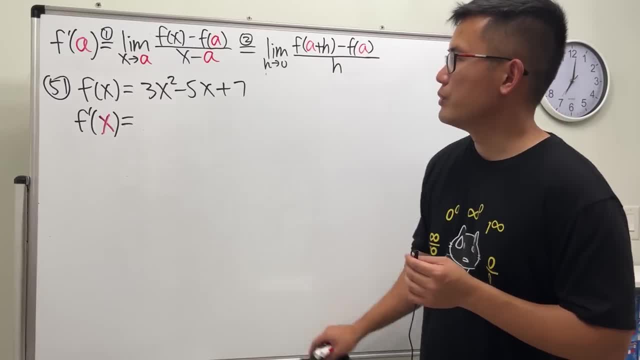 right. it does not look good at all, so no, right, it does not look good at all. so no, no, no, no, no, no, no. that's why we have definition two: if we want to do f prime of x, then we. if we want to do f prime of x, then we. 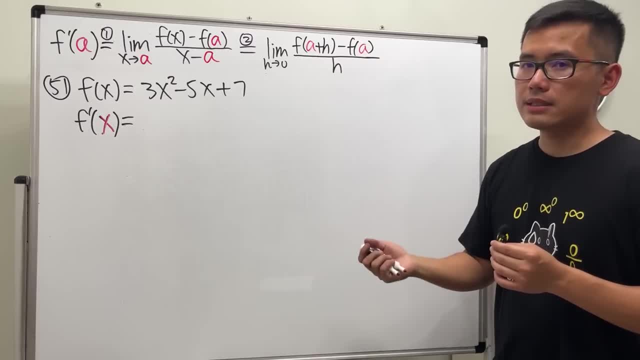 if we want to do f prime of x, then we look at this right here and just replace. look at this right here and just replace. look at this right here and just replace the a with x and then steal the jet. yeah, see, it's the official definition of. 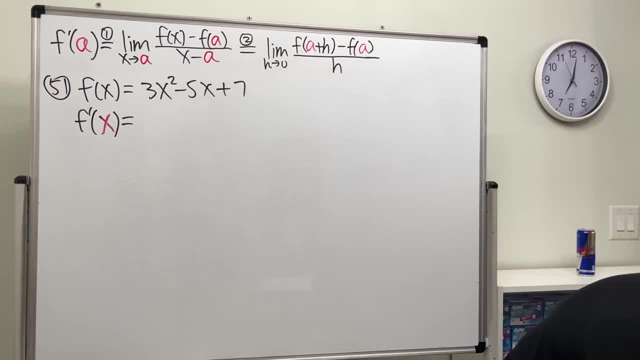 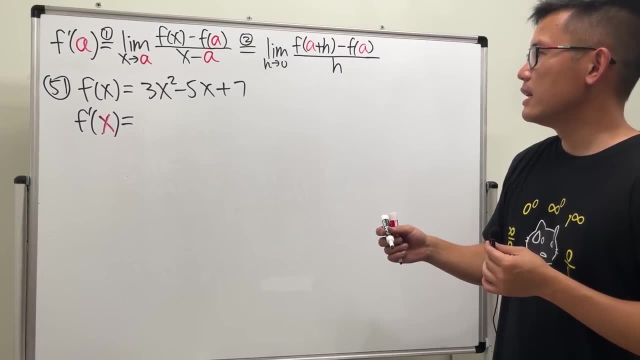 yeah, see, it's the official definition of. yeah, see, it's the official definition of the derivative. okay, so i am just going to. okay, so i am just going to okay, so i am just going to. hmm, now, i'm just going to write this right now, i'm just going to write this, right. 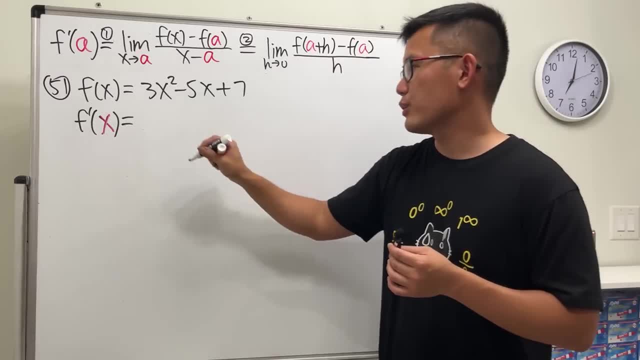 now i'm just going to write this right here: here we go, we're looking at here. here we go, we're looking at here. here we go, we're looking at definition two, and just change the a to definition two, and just change the a to definition two and just change the a to x. that's all you have to remember. so 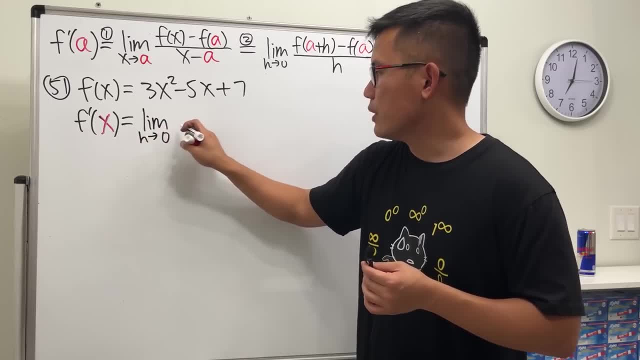 x, that's all you have to remember. so x, that's all you have to remember. so here we have the limit as h approaching. here we have the limit as h approaching. here we have the limit as h approaching zero. and this, right here, it's not zero and this, right here, it's not. 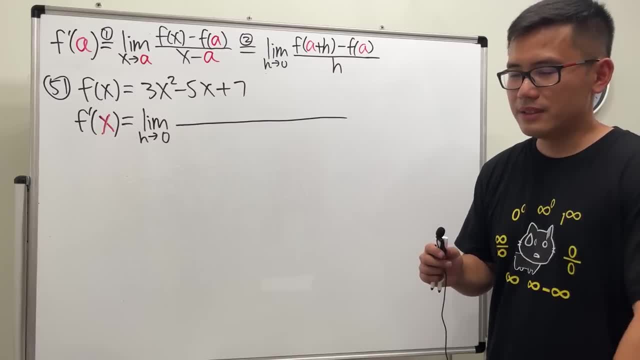 zero and this right here, it's not easy, easy, easy this is that perhaps the one of the this is that perhaps the one of the this is that perhaps the one of the first things that people first, things that people first, things that people dislike about the calculus part. 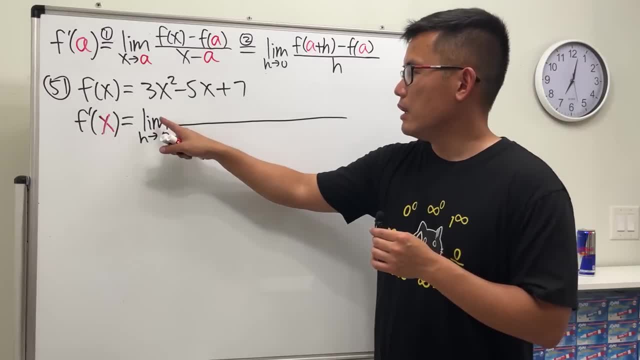 dislike about the calculus part. dislike about the calculus part is is is pretty demanding. i'll say pretty demanding. i'll say pretty demanding. i'll say anyway, anyway. anyway, we want to have f of x plus h, we want to have f of x plus h. we want to have f of x plus h. so what that means is: we want to look at. 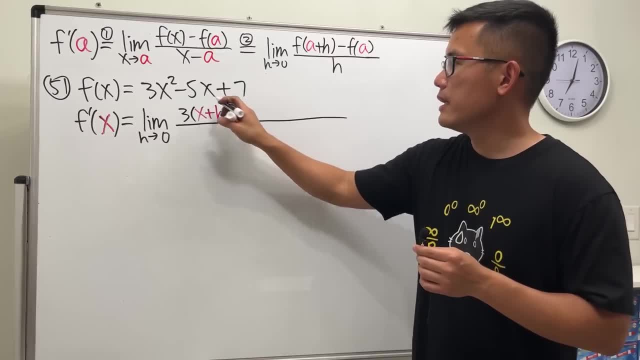 so what that means is: we want to look at. so what that means is we want to look at x plus h, x plus h, x plus h, and then square that, and then you continue, and then square that, and then you continue, and then square that, and then you continue minus f of. 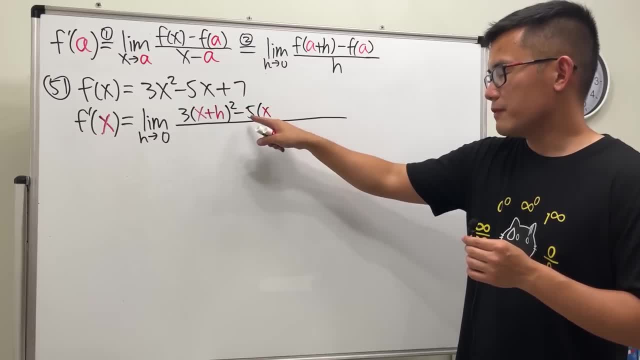 minus f of minus f of x, so minus five of x, so minus five of x, so minus five of minus five times x plus h, minus five times x plus h, minus five times x plus h, and then plus seven, so that's the f of, and then plus seven, so that's the f of. 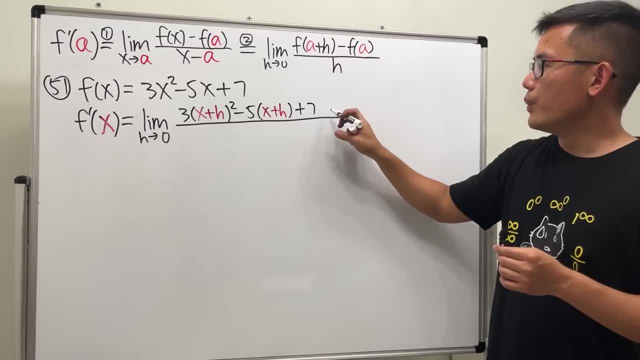 and then plus seven, so that's the f of x plus h part, x plus h part, x plus h part. and then we want to, and then we want to, and then we want to, minus f of x, which is just the original, minus f of x, which is just the original. 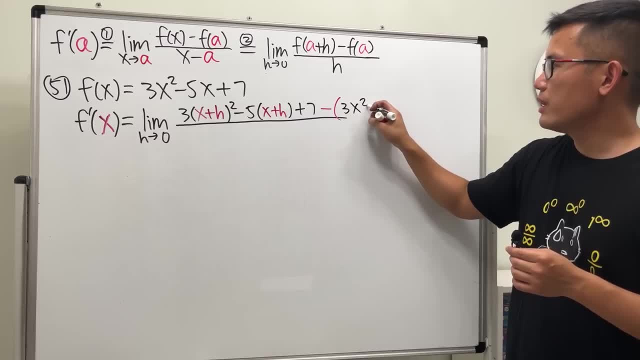 minus f of x, which is just the original. so just minus. and then we'll just put so just minus. and then we'll just put so just minus. and then we'll just put this down, this down, this down: 3x squared minus 5x plus 7.. 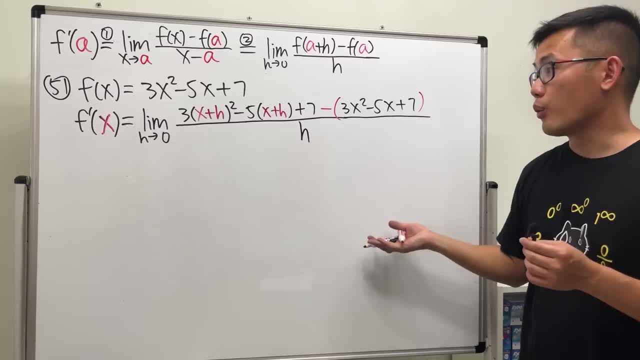 3x squared minus 5x plus 7.. 3x squared minus 5x plus 7.. and you can see that this expression is, and you can see that this expression is, and you can see that this expression is pretty long already, and 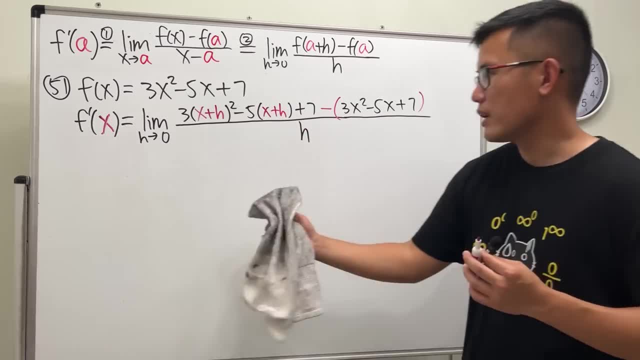 pretty long already and pretty long already and perhaps it's the longest, especially if perhaps it's the longest, especially if perhaps it's the longest, especially if you just come from, you just come from, you just come from pre-code and yeah, pretty intimidating so pre-code and yeah, pretty intimidating so. 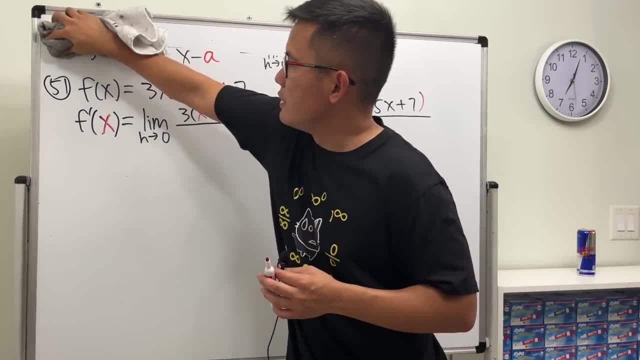 pre-code and yeah, pretty intimidating. so that's the idea, but for now i'm just that's the idea, but for now i'm just that's the idea, but for now i'm just going to erase both of this, so that way, going to erase both of this, so that way. 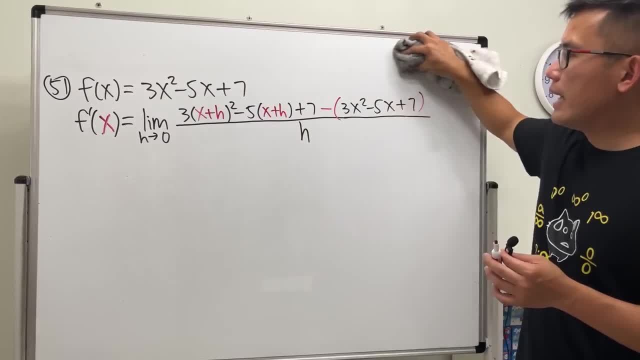 going to erase both of this. so that way we can, we can, we can actually just put down the definition of, actually just put down the definition of, actually just put down the definition of derivative for f, prime of x, derivative for f, prime of x, derivative for f- prime of x, and then we'll focus on that. so let me 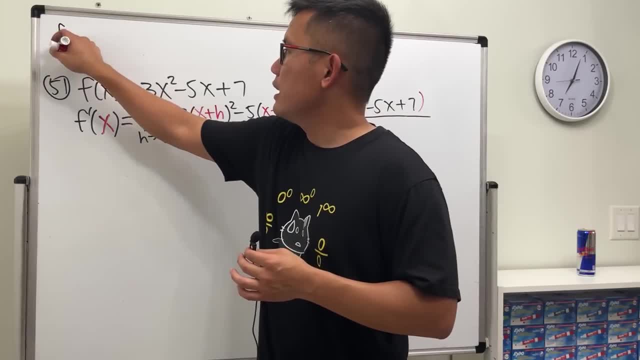 and then we'll focus on that. so let me, and then we'll focus on that. so let me do that for you guys right here, do that for you guys right here, do that for you guys right here. so, ladies and gentlemen, f prime of x. so, ladies and gentlemen, f prime of x. 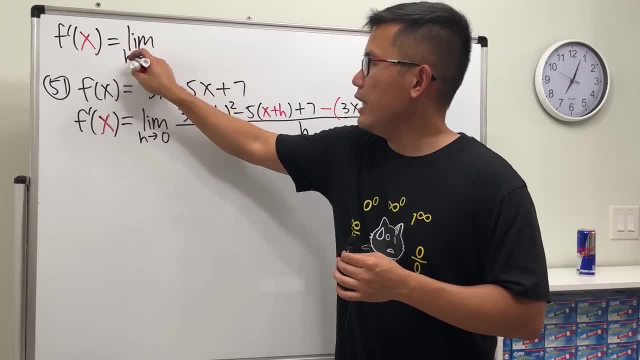 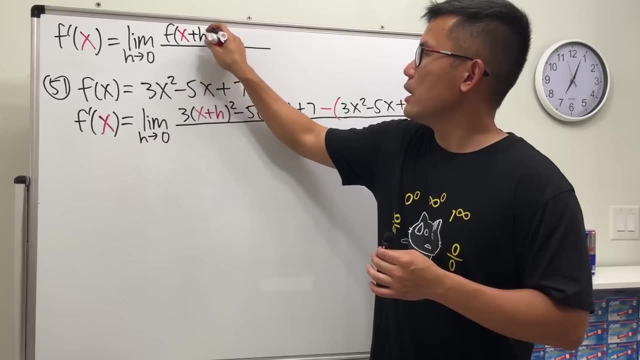 so, ladies and gentlemen, f- prime of x. this, right here, equals the limit as h. this right here equals the limit as h. this right here equals the limit as h approaching zero, approaching zero, approaching zero. we have f of x plus h. we have f of x plus h. 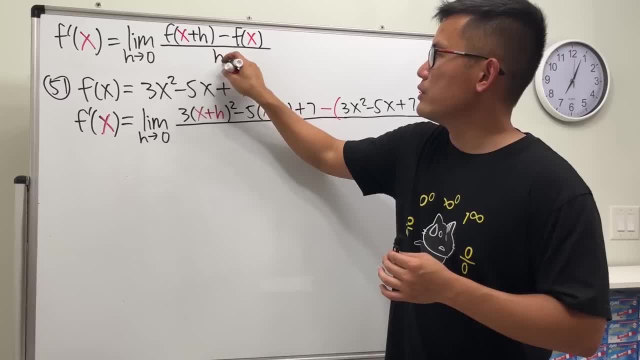 we have f of x plus h minus f of x minus f of x minus f of x, and then over h, and then over h, and then over h, and this is definitely, and this is definitely, and this is definitely a definition that you have to remember, a definition that you have to remember. 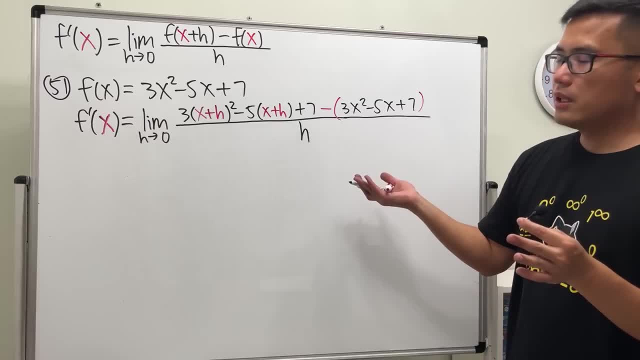 a definition that you have to remember for your calculus class, for your calculus class, for your calculus class. so how do we take off this? so how do we take off this? so how do we take off this? well, we will have to expand it, that's. well, we will have to expand it, that's. 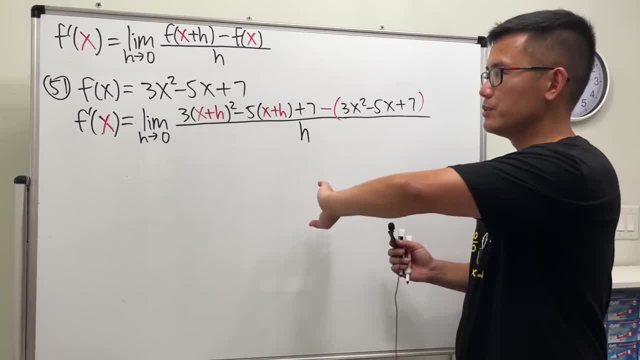 well, we will have to expand it. that's what i told you guys earlier. i just what i told you guys earlier. i just what i told you guys earlier. i just used definition one because now we will used definition one, because now we will used definition one, because now we will just be doing this right here. 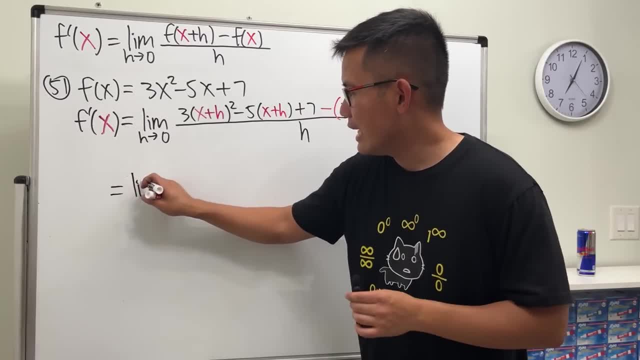 just do it all right, here we go this. just do it all right, here we go this. just do it all right. here we go this. right here we have the limit as h. right here we have the limit as h. right here we have the limit as h approaching zero. 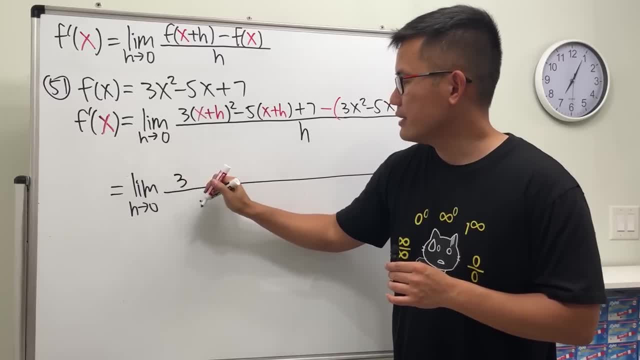 open this, we get open this, we get open this, we get three in the front, and then we have three in the front, and then we have three in the front, and then we have- let's just put this down in black x. let's just put this down in black x. 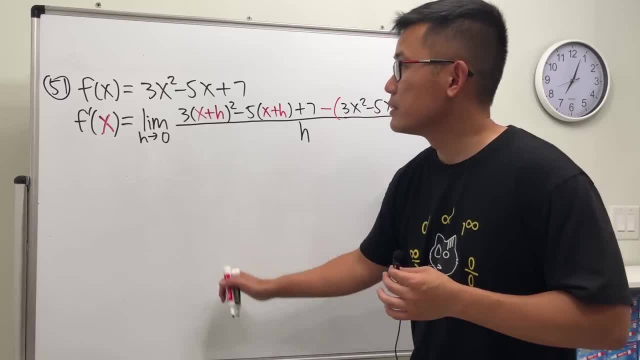 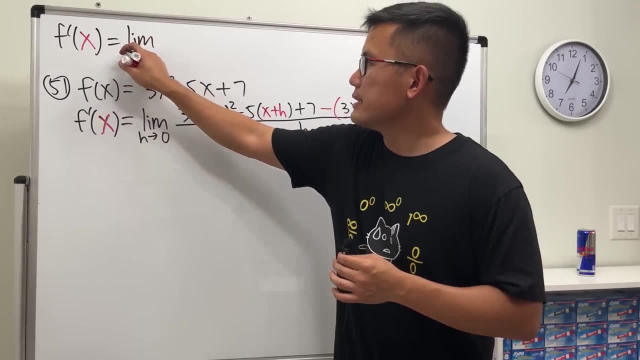 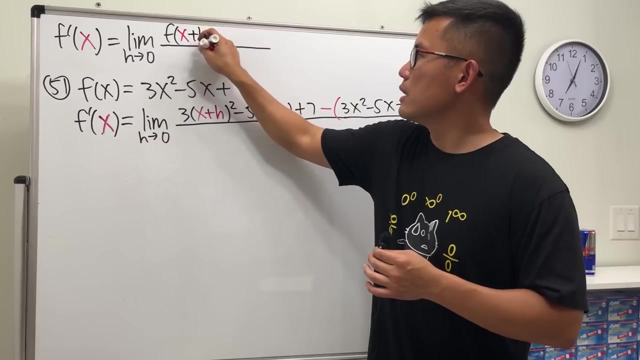 on that. So let me do that for you guys right here. So, ladies and gentlemen, f prime of x, This right here equals the limit as h approaching 0. We have f of x plus h, minus f of x, and then all over h. 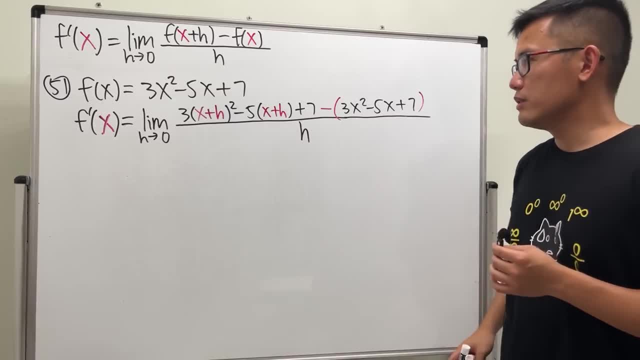 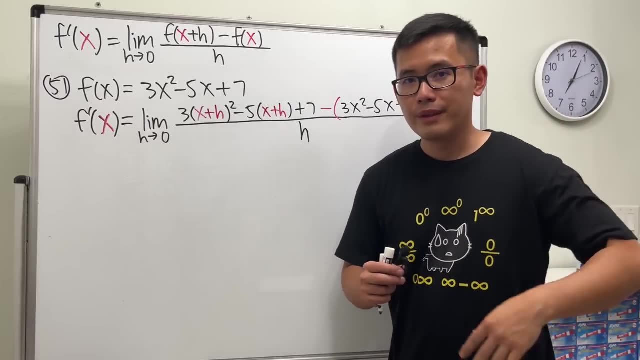 And this is definitely a definition that you have to remember for your calculus class. So how do we take off this? Well, we will have to expand it. That's why I told you guys earlier, I just used definition 1, because now we will. 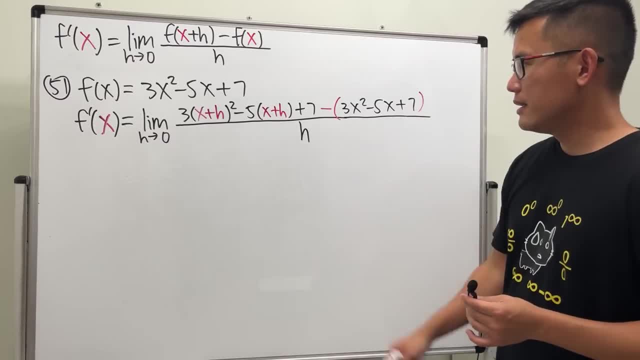 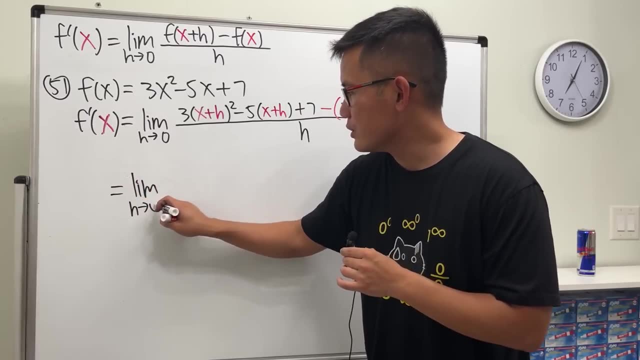 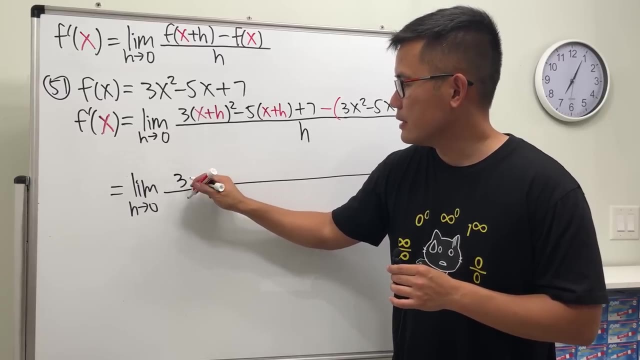 just be doing this right here. Just do it. Alright, here we go This right here. we have the limit as h approaching 0. Open this, we get 3 in the front, and then we have- let's just put this down in black. 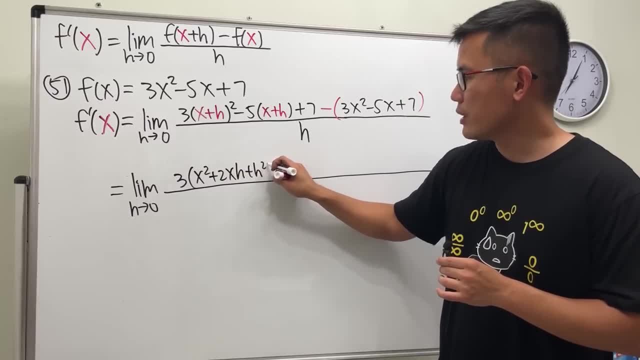 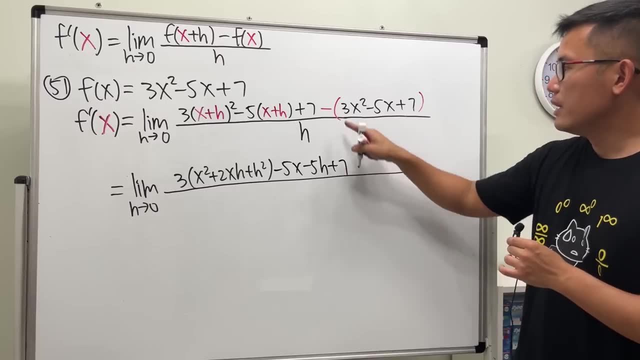 x squared plus 2xh, And then plus h squared, And then distribute it, we get minus 5x minus 5h, And then this is the plus 7.. Distribute it, we get negative 3x squared minus minus. 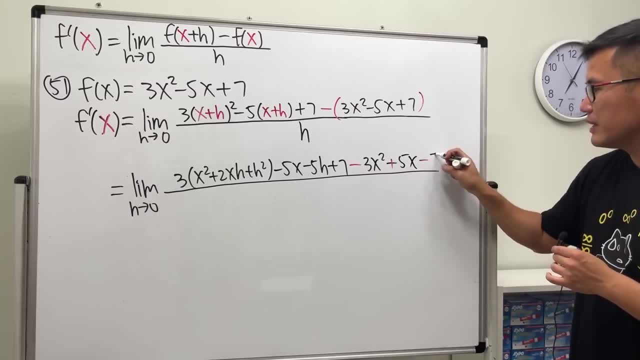 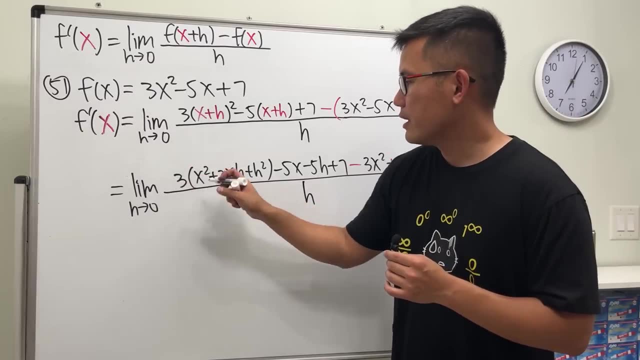 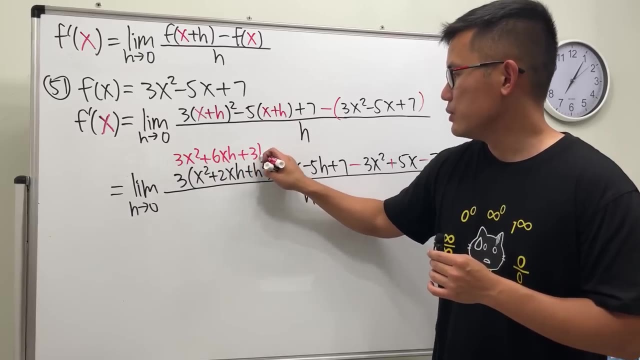 becomes plus 5x and then minus 7.. And then all over h. But don't forget, we still have this to be distributed. Let me just put it on the top. Here we have 3x squared plus 6xh and then plus 3h. 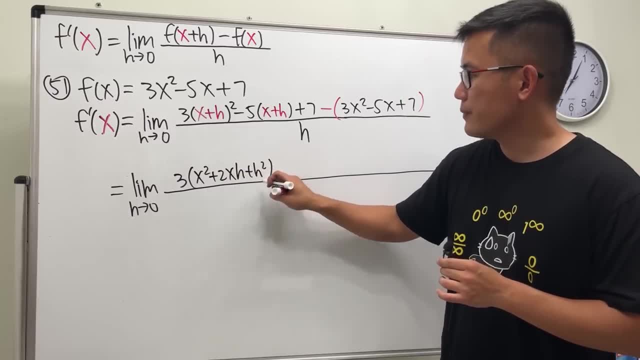 let's just put this down in black: x square plus 2x h, and then plus h square plus 2x h, and then plus h square plus 2x h, and then plus h square, square, square, and then distribute it. we get minus 5x. 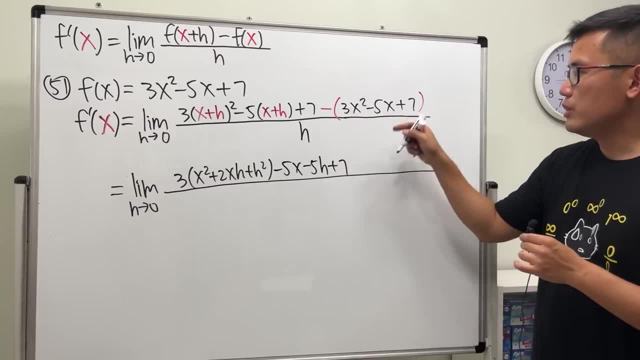 and then distribute it: we get minus 5x. and then distribute it: we get minus 5x minus 5h. and then this is the plus 7 minus 5h, and then this is the plus 7 minus 5h, and then this is the plus 7. distribute: we get negative 3x squared. 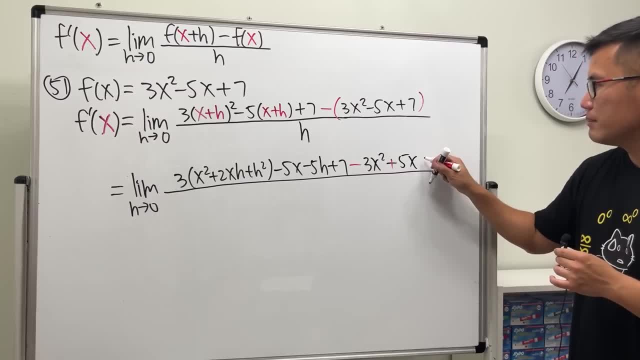 distribute: we get negative 3x squared. distribute: we get negative 3x squared. minus minus becomes plus. minus minus becomes plus. minus minus becomes plus 5x and then minus 7, 5x, and then minus 7, 5x and then minus 7 and then over h. and then over h, and then over h, but don't forget, we still have this to. but don't forget, we still have this to. but don't forget, we still have this to to be distributed. let me just put it on to be distributed. let me just put it on. 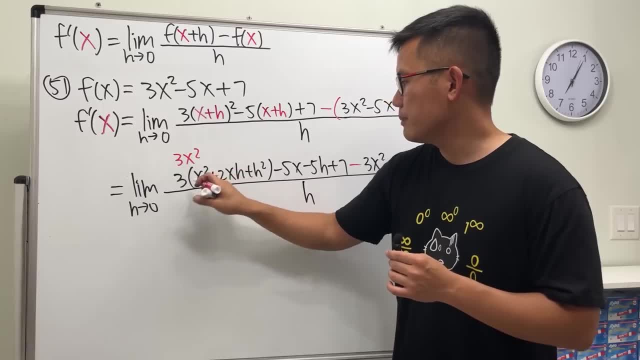 to be distributed. let me just put it on the top. here we have the top. here we have the top. here we have 3x squared plus 3x squared, plus 3x squared, plus 6x h, and then plus 3h squared, 6x h, and then plus 3h squared. 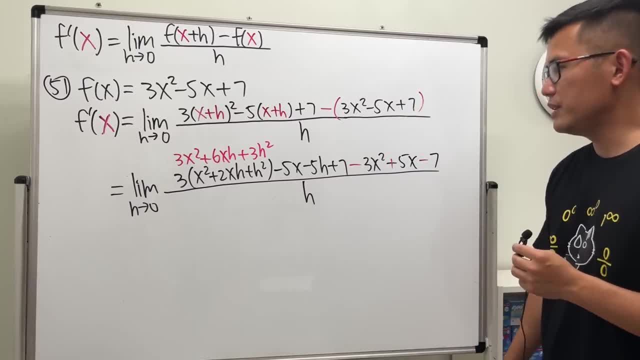 6x h and then plus 3h squared. now, here's the best part we can cancel now. here's the best part we can cancel now, here's the best part we can cancel. things, things, things. hopefully, let's see, hopefully, let's see, hopefully, let's see 3x squared. 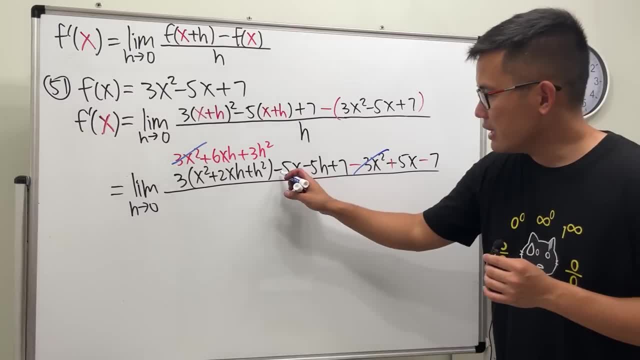 3x squared- 3x squared negative. 3x squared: cancel good. negative. 3x squared: cancel good. negative. 3x squared: cancel good. negative. 5x negative. 5x negative. 5x positive. 5x cancel good. positive. 5x cancel good. 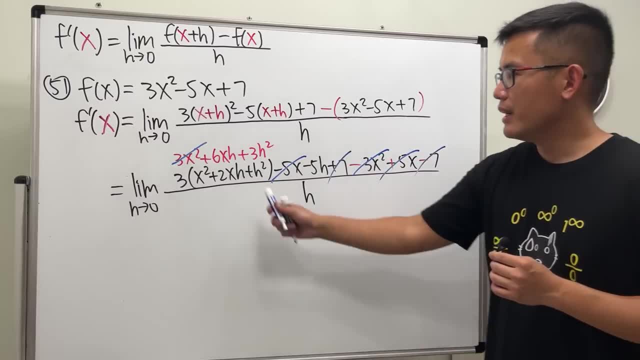 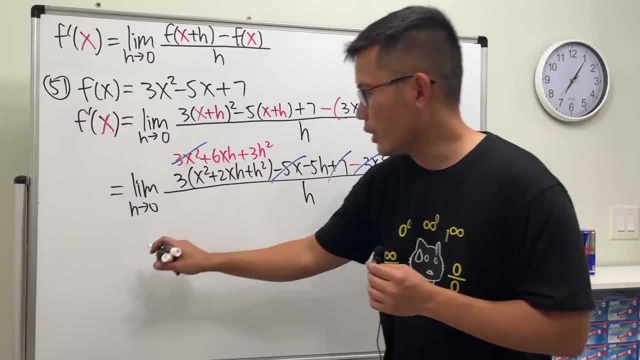 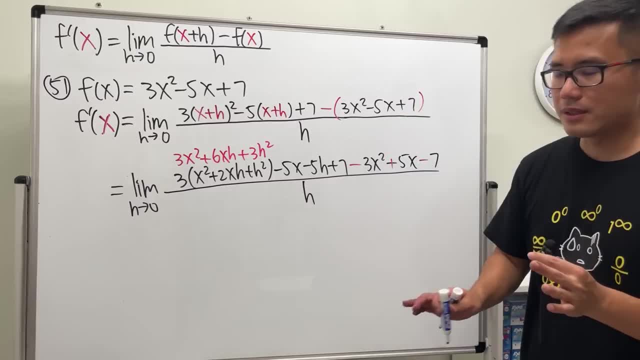 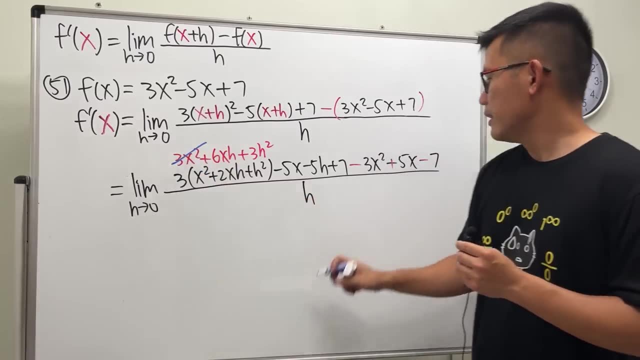 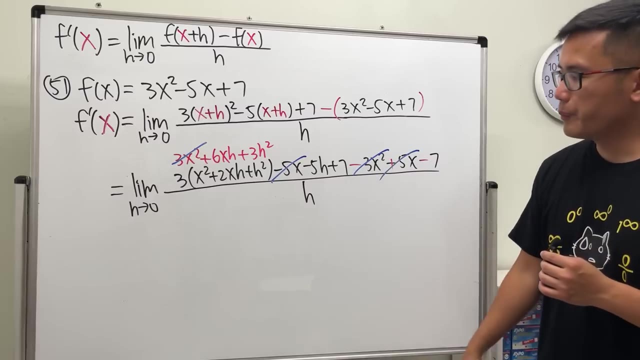 squared. Now here's the best part: We can cancel things. hopefully Let's see: 3x squared negative, 3x squared cancel good, Negative. 5x positive. 5x cancel good, 7 minus 7. 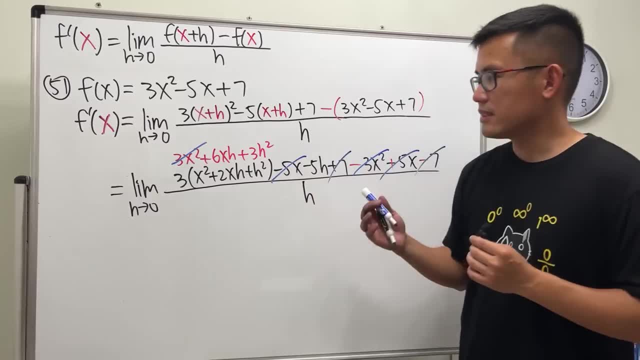 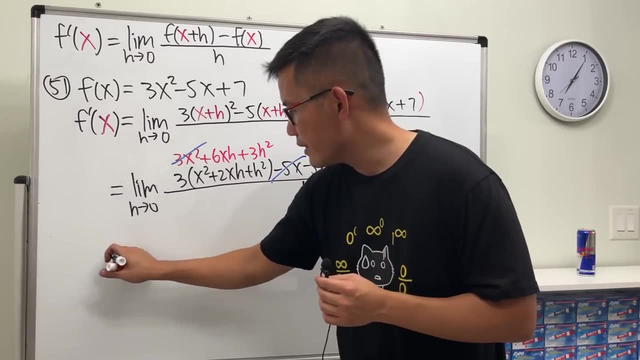 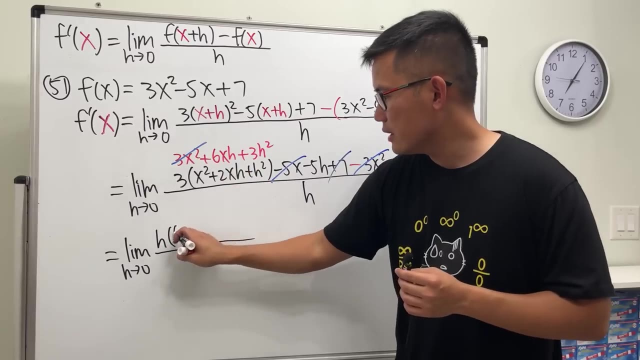 no more good. This, this and that remains on the top. And notice, everybody has an h. We can factor that out, So we will. Here we have the limit as h approaching 0.. Factor out the h We get first thing. 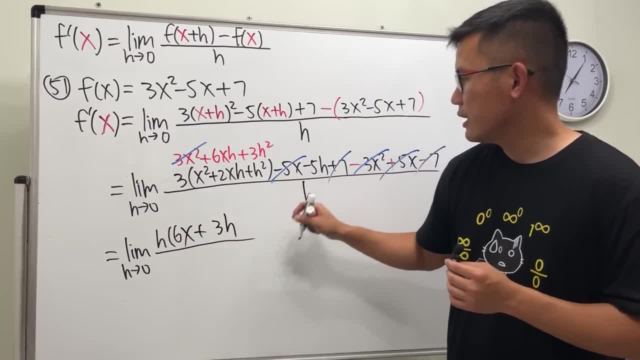 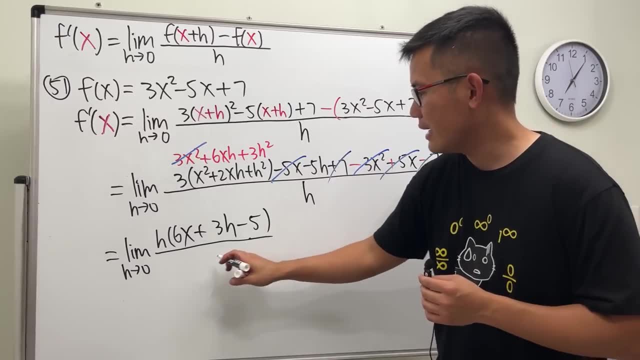 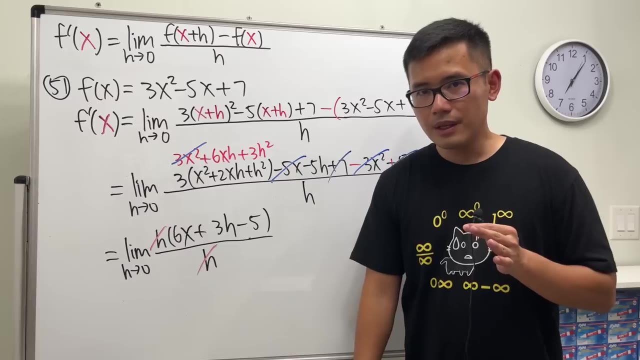 6x. second thing plus 3h and the last thing, right here, we have the minus 5.. Don't forget, we still have this remained. And then all divided by h, Now cancel out the h, And this is the reason why I told you, guys, you should keep. 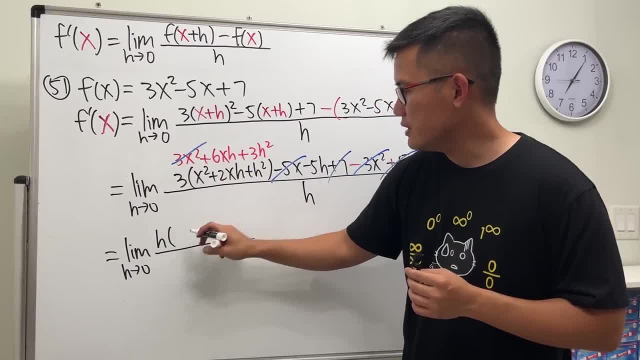 here we have the limit as h approaching zero, zero, zero. factor out the h, we get first thing 6x. factor out the h, we get first thing 6x. factor out the h, we get first thing 6x. second thing, second thing, second thing, plus 3h and the last thing right here. 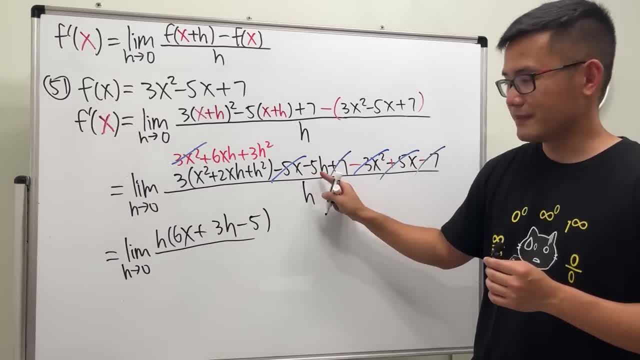 plus 3h and the last thing right here: plus 3h. and the last thing right here, we have the minus five, we have the minus five, we have the minus five. don't forget to have this remained, don't forget to have this remained, don't forget to have this remained. and then, all divided by h: 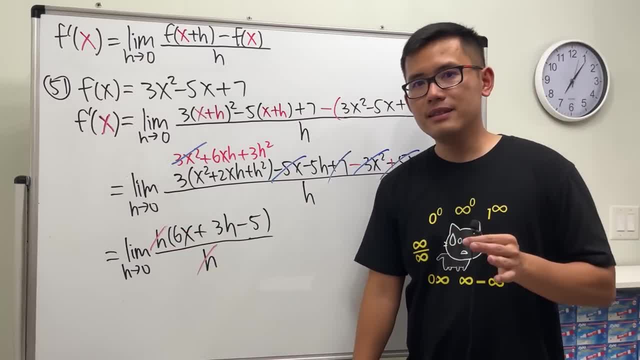 and then all divided by h and then all divided by h. now cancel out the h and this is the. now cancel out the h and this is the. now cancel out the h. and this is the reason why i told you guys you should reason why i told you guys you should. 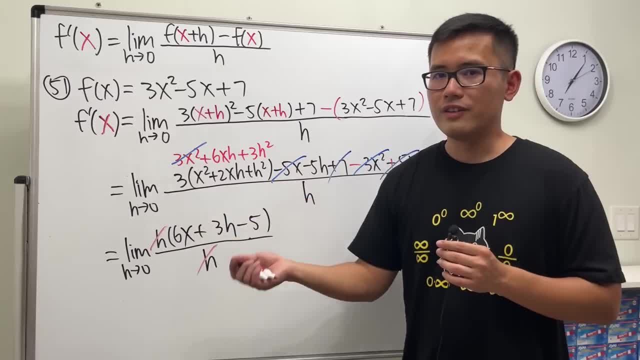 reason why i told you, guys you should keep writing down the limit as h, keep writing down the limit as h, keep writing down the limit as h approaching zero, or like whatever is approaching zero, or like whatever is approaching zero, or like whatever is approaching whatever. because now you see, 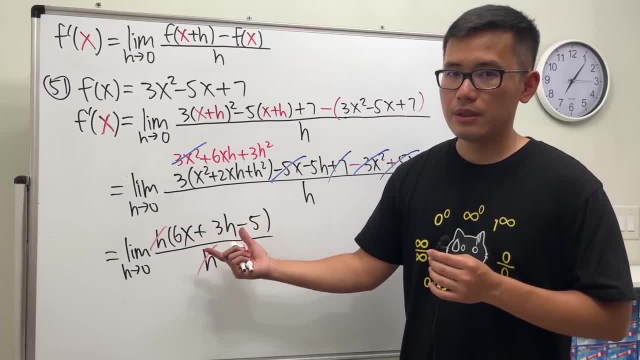 approaching whatever. because now you see approaching whatever, because now you see how, how, how we have both x and h in the expression. we have both x and h in the expression. we have both x and h in the expression, but it's only h is approaching zero. so 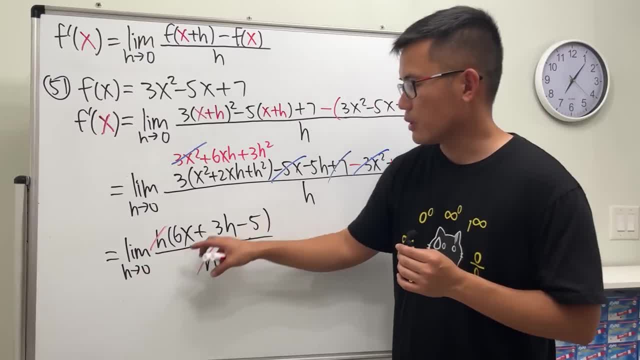 but it's only h is approaching zero. so, but it's only h is approaching zero. so you're plugging zero into h, you're plugging zero into h, you're plugging zero into h. so this is second reminder, what you have. so this is second reminder, what you have. 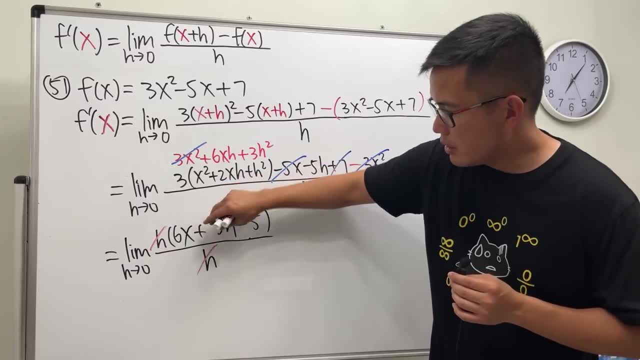 so this is second reminder, what you have to do, to do, to do you put h to be zero in here, so you just you put h to be zero in here, so you just you put h to be zero in here, so you just have 6x. 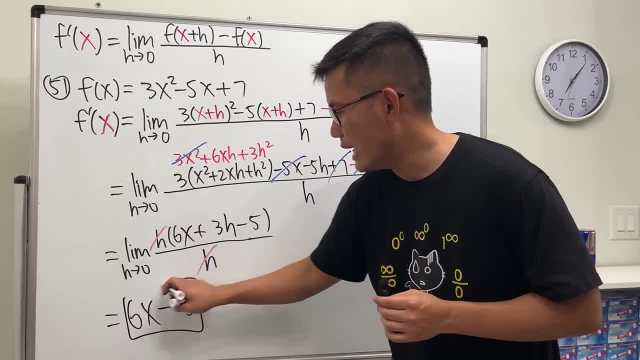 no more, and then minus 5. and here you no more, and then minus 5, and here you no more, and then minus 5. and here you have it. that's the answer. have it, that's the answer, have it. that's the answer. can we do this in five seconds? yes, 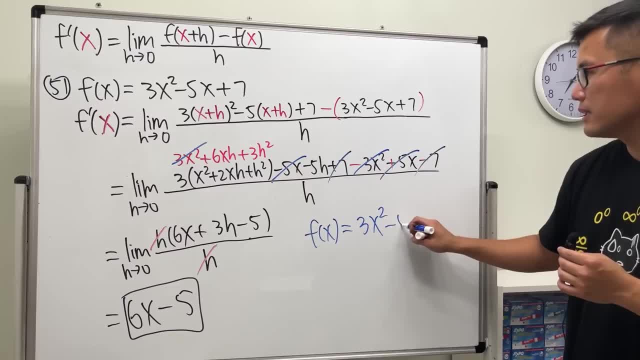 can we do this in five seconds? yes, can we do this in five seconds? yes. f of x equals 3x squared minus 5x. f of x equals 3x squared minus 5x. f of x equals 3x squared minus 5x, plus 7 derivative. 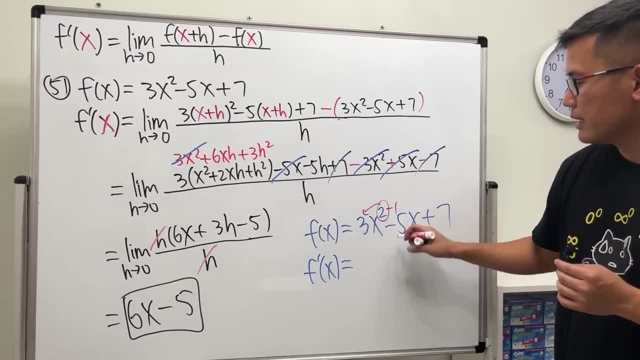 plus 7 derivative. plus 7 derivative. in action, in action, in action. power rule: bring the power to the front. power rule: bring the power to the front. power rule: bring the power to the front. minus one six x to the first power, minus one six x to the first power. 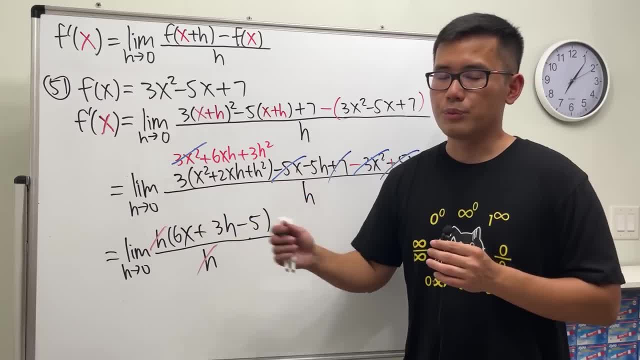 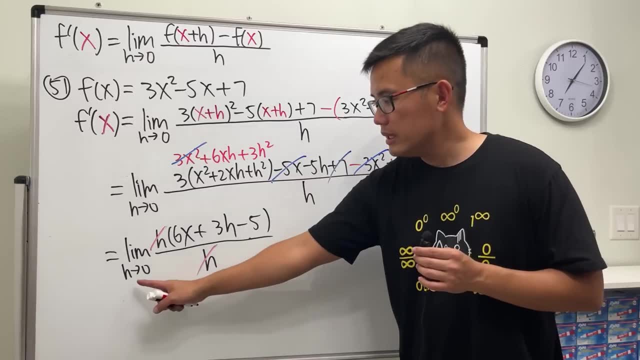 writing down the limit as h approaching 0 or like whatever is approaching whatever, because now you see how we have both x and h in the expression, but it's only h is approaching 0, so you're plugging 0 into h. So this is a good reminder of what 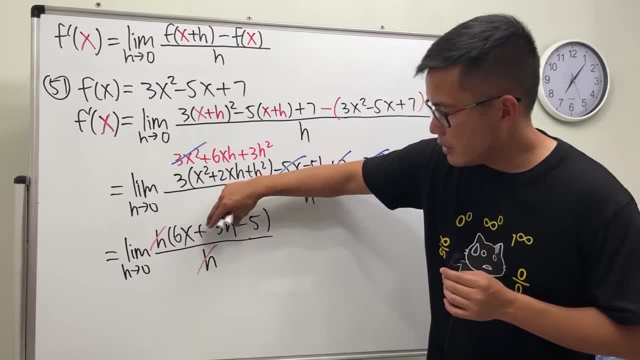 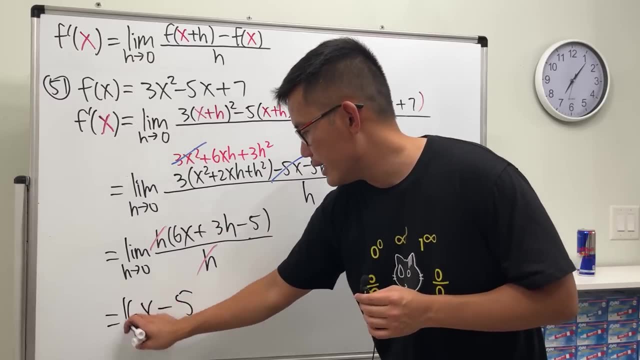 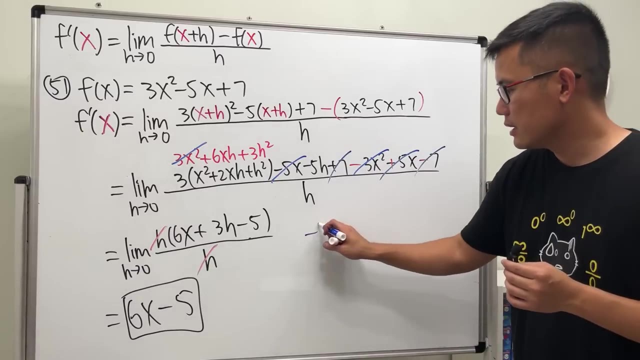 you have to do. You put h to be 0 in here, so you just have 6x, no more, and then minus 5.. And here you have it. That's the answer. Can we do this in 5 seconds? Yes, 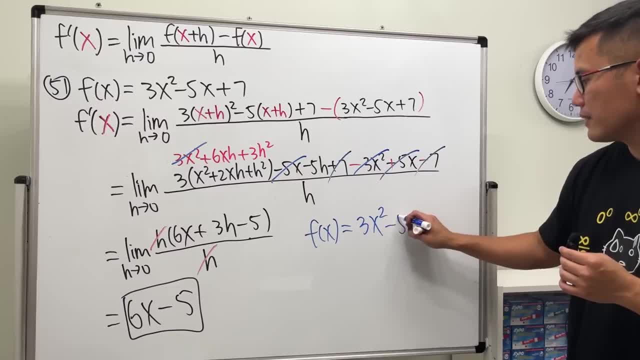 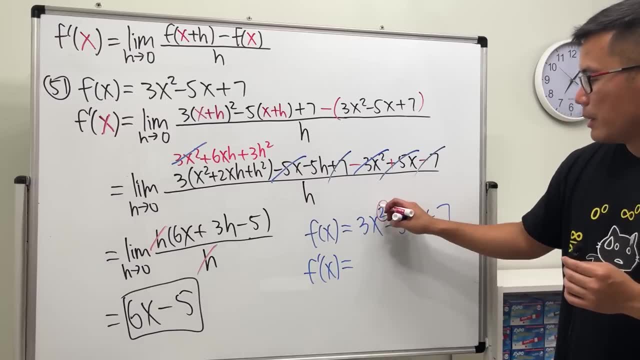 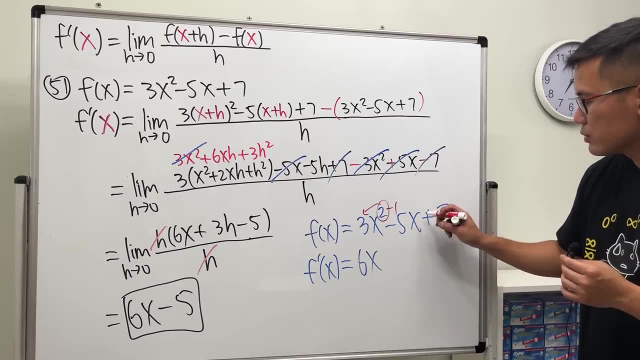 f of x equals 3x squared minus 5x plus 7. derivative in action Power rule: Bring the power to the front. minus 1. 6x to the first power. Second part: Minus 5x to the first power. 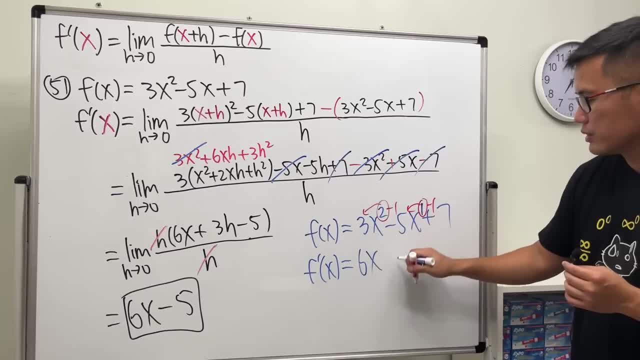 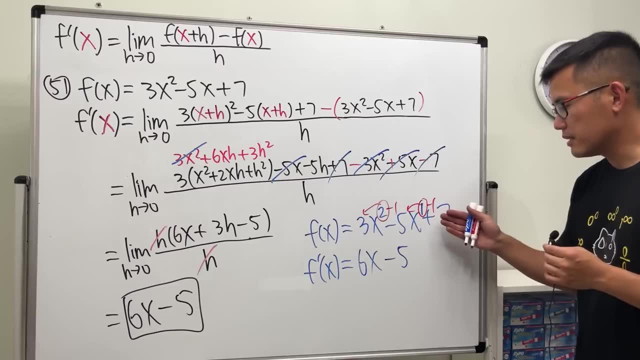 Bring the power to the front. minus 1.. So just minus 5.. x plus 0,, just 1.. This is a good, This right here. No x, So it's just a constant. The derivative of this is just 0.. 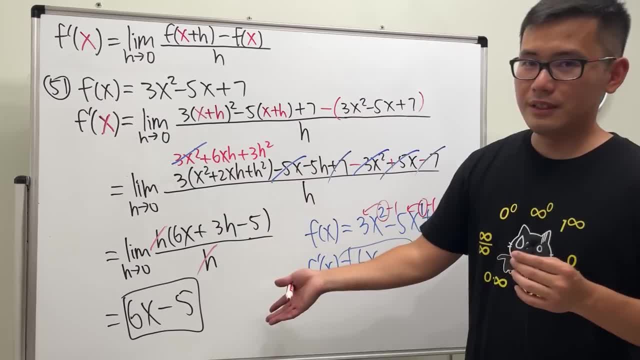 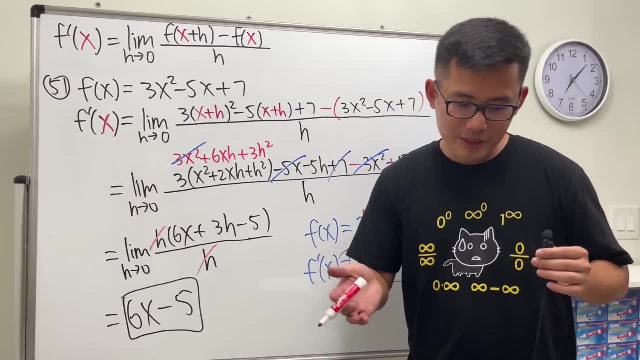 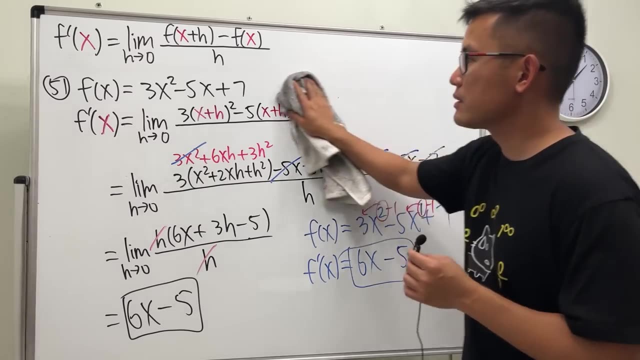 So done. I know, I know, I know Why are we doing this. You will see, Let's practice one more and then you will see For 53,, 54,, 55. then you will really see why we need the definition of derivative. 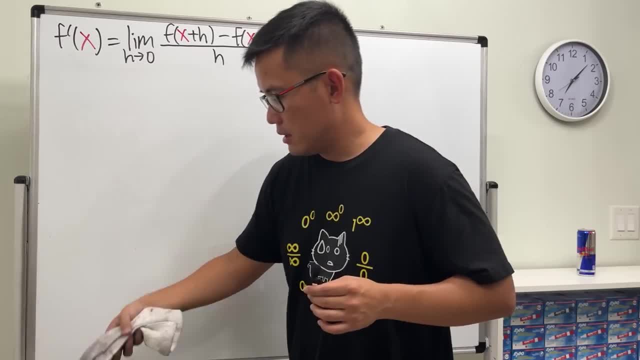 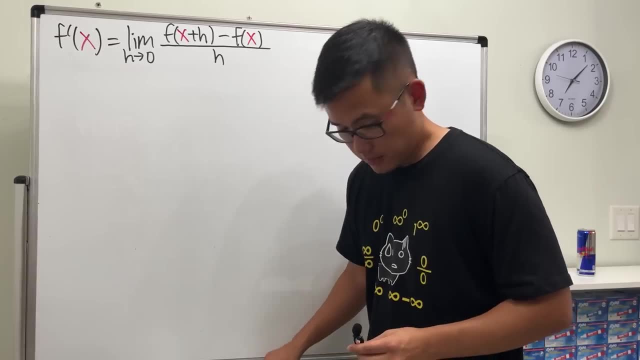 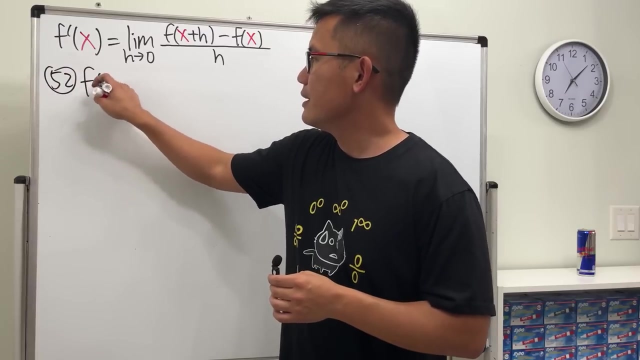 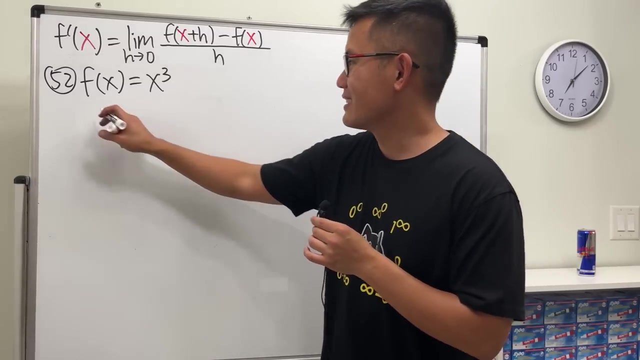 Let me just check. Very good 52. It's a very simple function. It's just x to the third power. I didn't want to go too crazy. We want the f prime of x, So here we go. Okay, Let me just put it down like this: 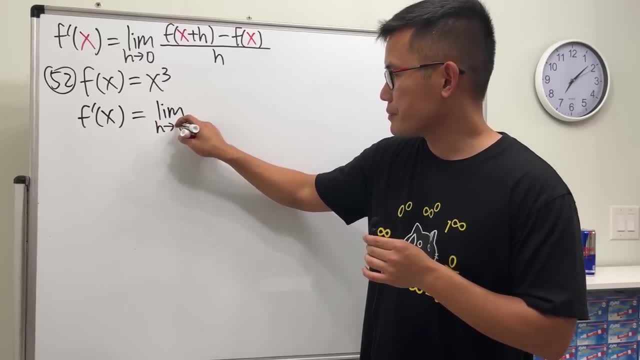 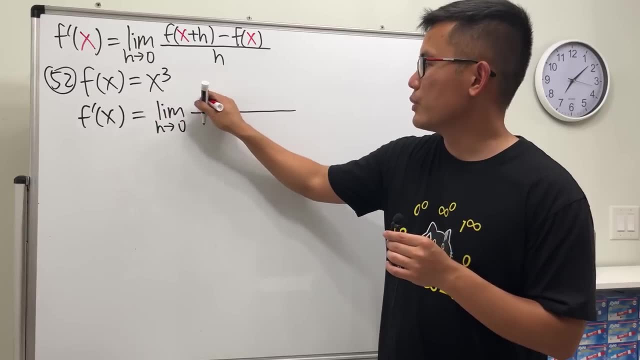 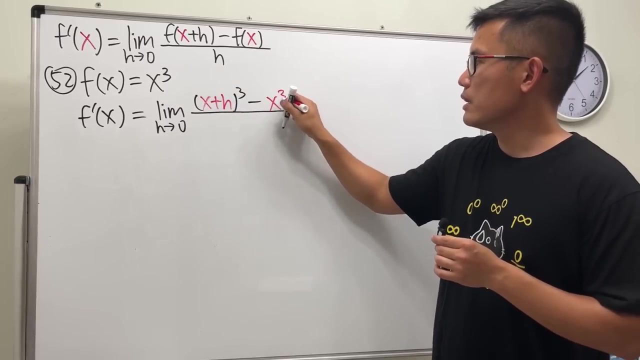 So here we go. We want the limit as x as h, approaching 0.. And then this part means we're just plugging x plus h into here. So we have x plus h, third power, and then minus f of x, which is just that original. 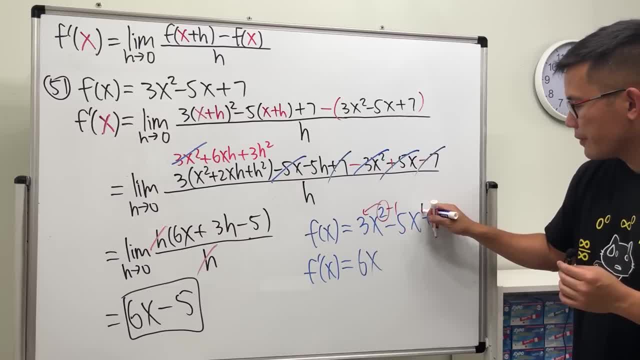 minus one six x to the first power second part. minus five x to the first second part. minus five x to the first second part. minus five x to the first power. yeah, power, yeah, power, yeah. bring the power to the front minus one. bring the power to the front minus one. 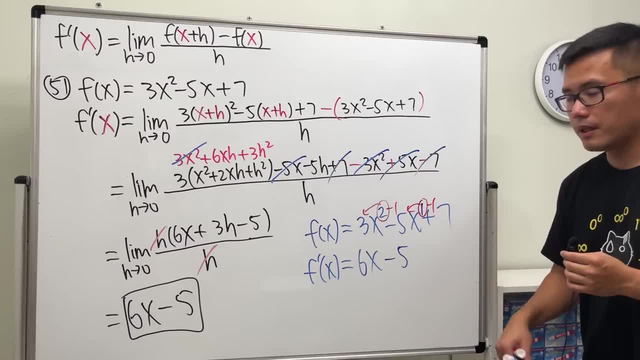 bring the power to the front. minus one, so just minus five x plus zero, so just minus five x plus zero, so just minus five x plus zero. just one, just one, just one. this right here, no x, so it's just a. this right here, no x, so it's just a. 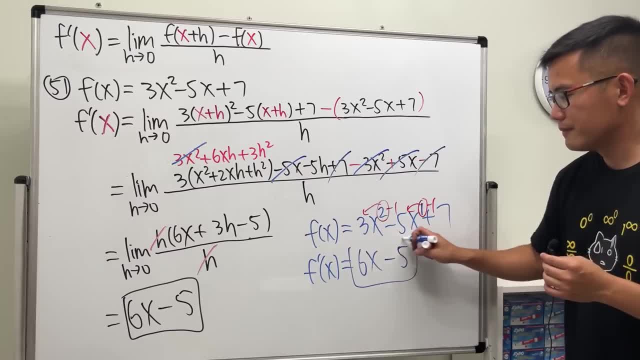 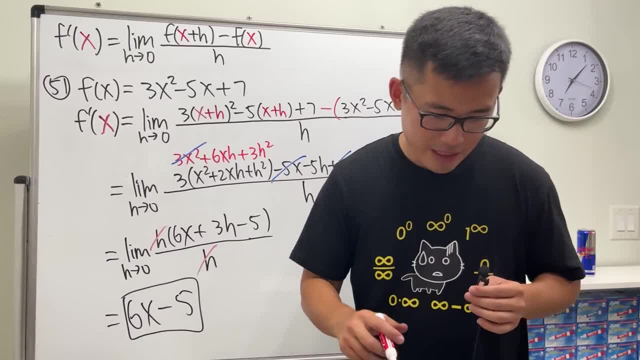 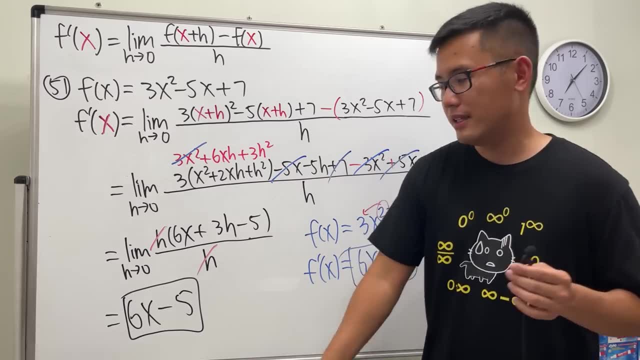 i know, i know, i know why are we doing this, why are we doing this, why are we doing this? you'll see, let's, you'll see, let's, you'll see, let's uh, practice one more, and then uh, practice one more, and then uh, practice one more, and then you'll see, for 53, 54, 55, then you. 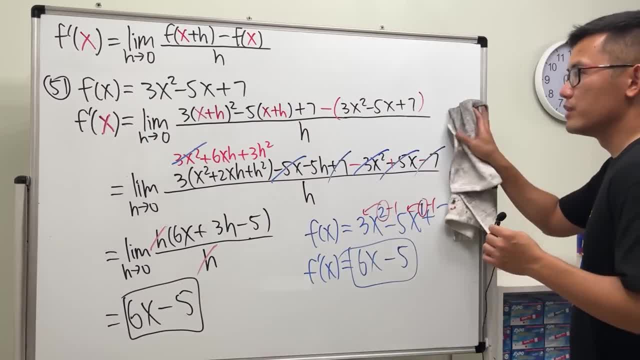 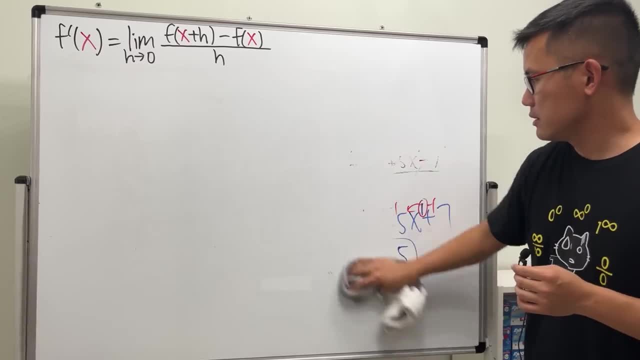 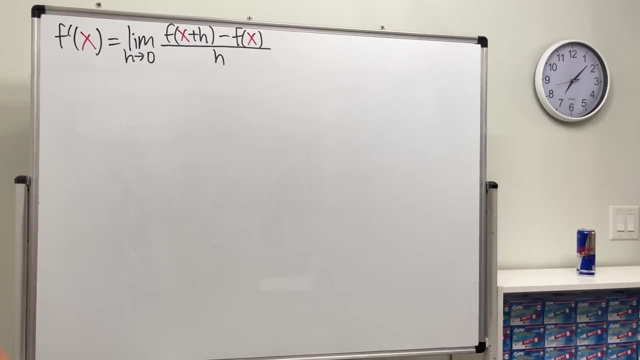 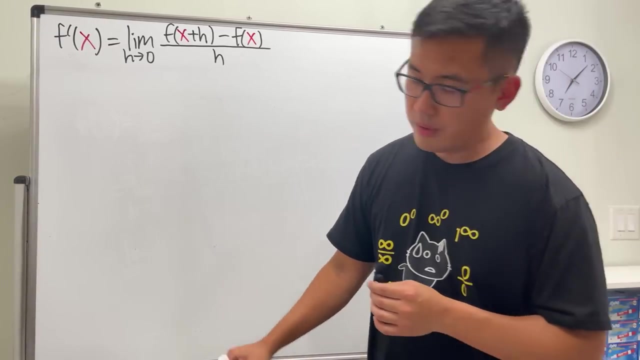 you'll see for 53, 54, 55, then you you'll see for 53, 54, 55, then you already see why, already see why already see why we need the definition of derivative. we just check, we just check, we just check. very good, 52.. 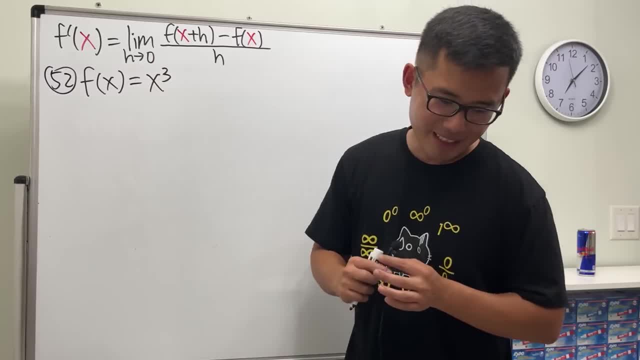 it's a very simple function. it's just x. it's a very simple function, it's just x. it's a very simple function. it's just x to third power. i didn't want to go too to third power. i didn't want to go too to third power. i didn't want to go too crazy. we want the f prime of x. so here: 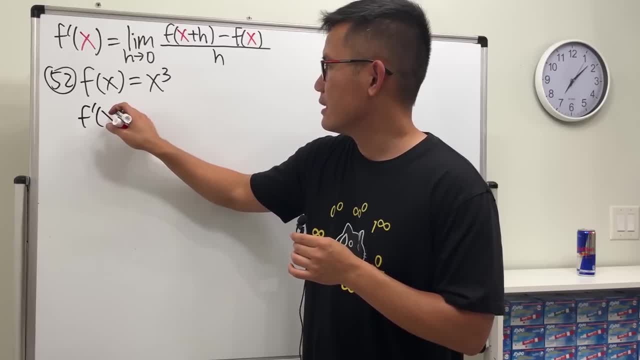 crazy, we want the f prime of x. so here, crazy, we want the f prime of x. so here we go: f prime of x, we go f prime of x, we go f prime of x. okay, let me just put it down like this: so okay, let me just put it down like this: so: 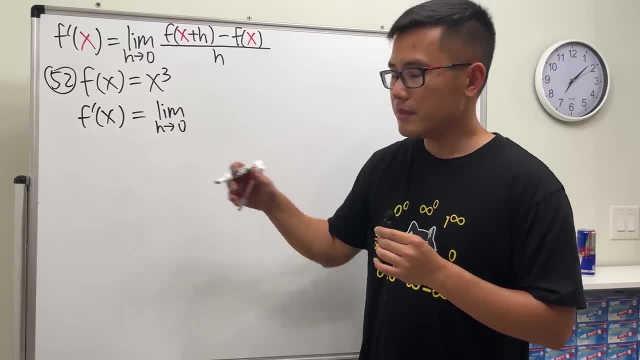 okay, let me just put it down like this: so here we go, we want the limit as x. here we go. we want the limit as x, here we go. we want the limit as x, as h approaching zero, and then as h approaching zero, and then as h approaching zero, and then this part means we're just plugging x. 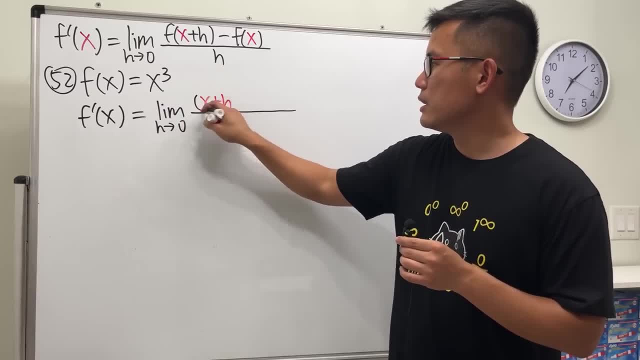 this part means we're just plugging x. this part means we're just plugging x plus h into here, so we have x plus h plus h into here. so we have x plus h plus h into here, so we have x plus h, third power, and then minus f of x, which 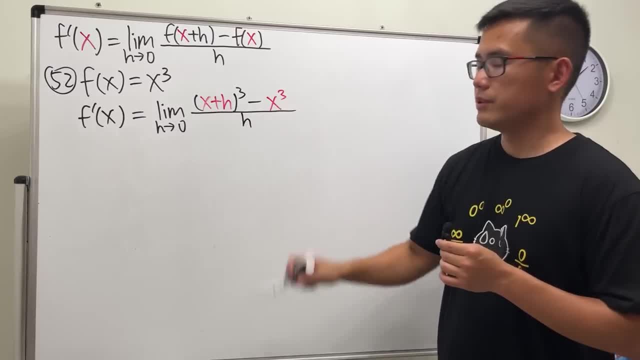 third power, and then minus f of x, which third power. and then minus f of x, which is just that original is just that original is just that original. and then o over h, and then o over h, and then o over h. open this, open this. open this, we get. 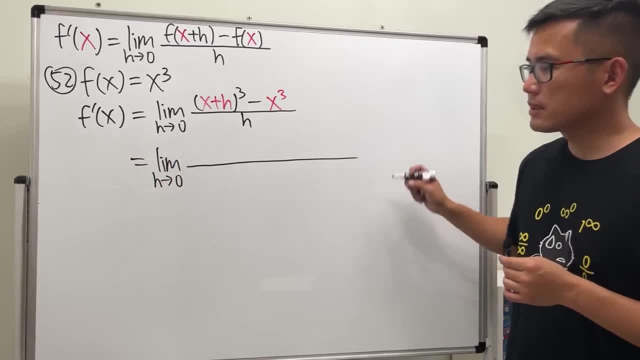 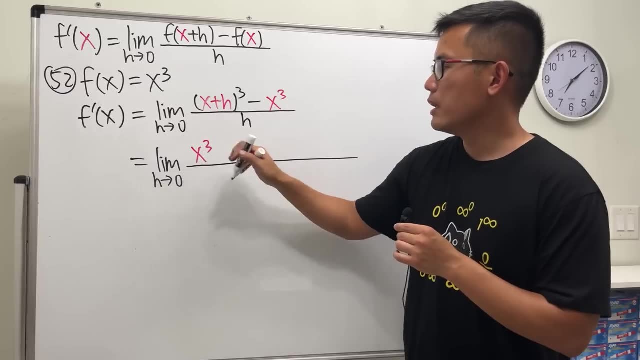 we get. we get limit as h approaching zero, and let's use limit as h approaching zero, and let's use limit as h approaching zero and let's use the pascal triangle, the pascal triangle, the pascal triangle plus, three times x square and h to the. 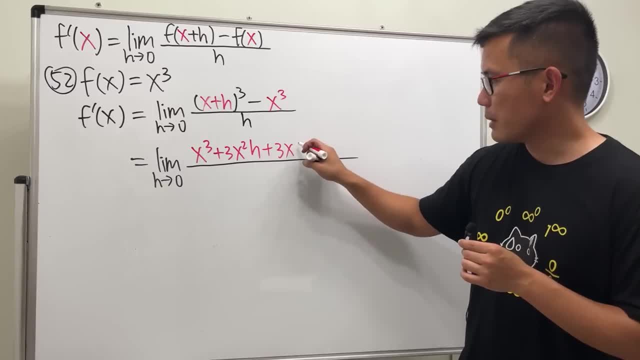 plus three times x square and h to the plus three times x square and h to the first power. first power, first power. and then plus three times x to the first, and then plus three times x to the first, and then plus three times x to the first power: h square. 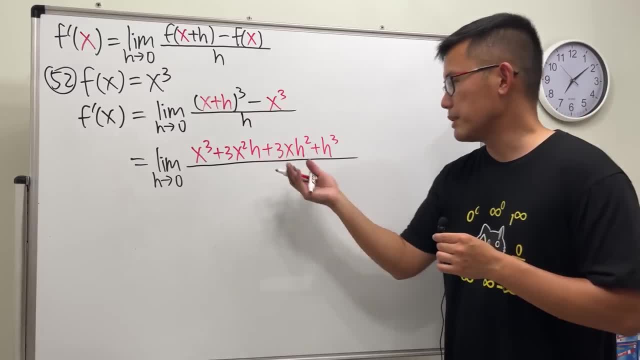 power. h square power. h square plus h to the third power, plus h to the third power, plus h to the third power. that's the expansion for that, and then that's the expansion for that, and then that's the expansion for that, and then minus x to the third power. o of h. 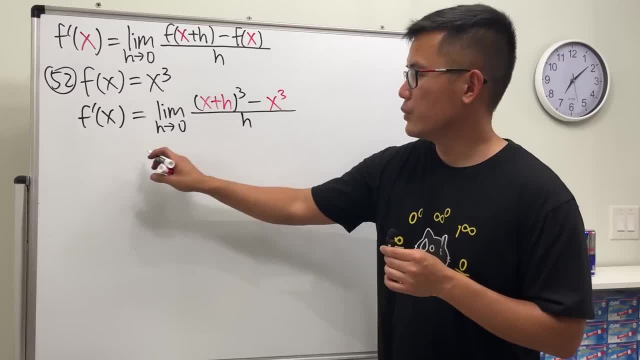 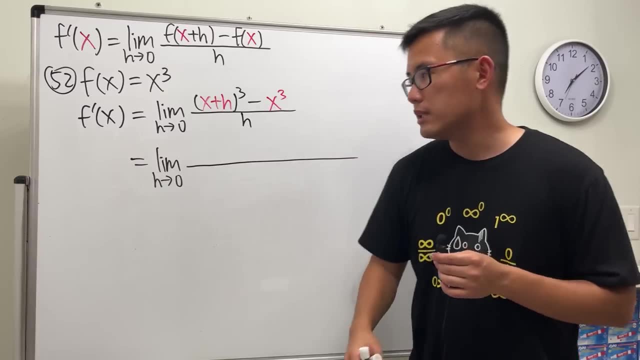 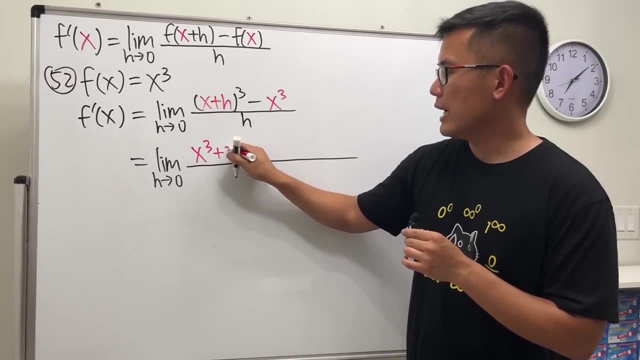 and then 0 over h. Open this, We get limit as h approaching 0.. And let's use the Pascal Triangle. So first we will have 1 times x to the third power, so just x to the third power plus 3 times. 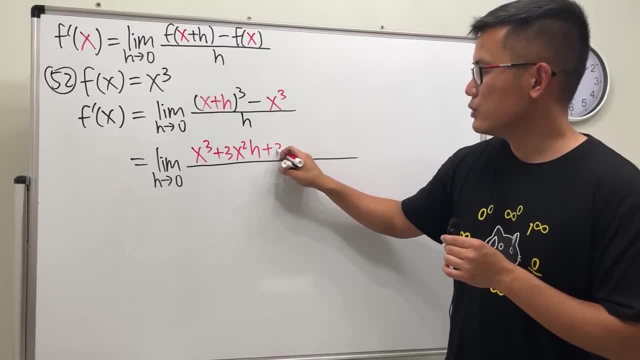 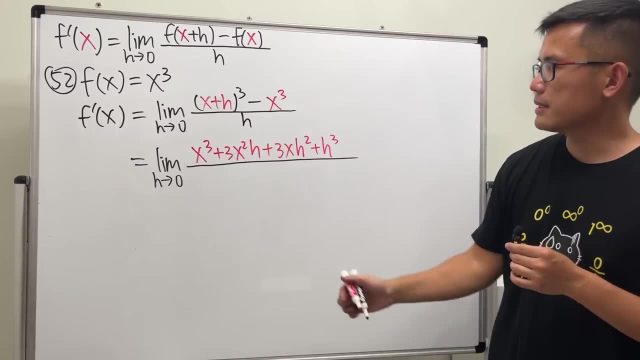 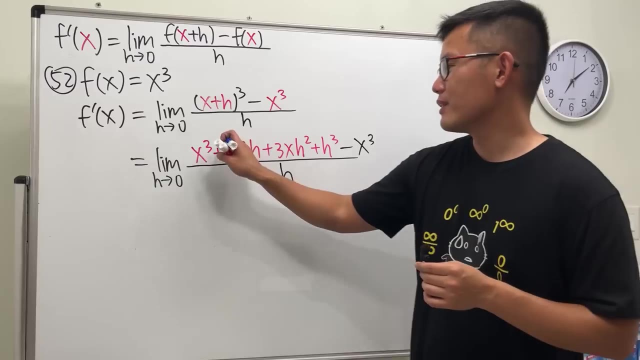 x squared and h to the first power, and then plus 3 times x to the first power, h squared, plus h to the third power, That's the expansion for that. And then minus x to the third power, 0 over h. We can only cancel one thing. 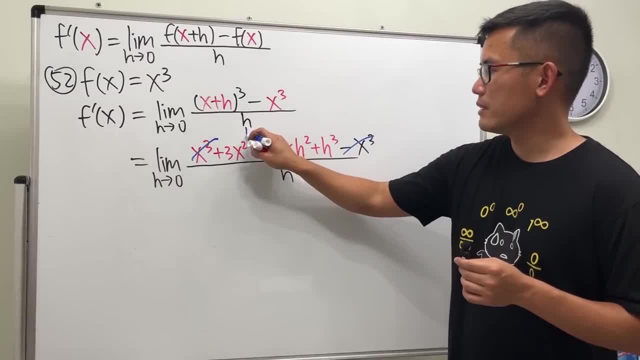 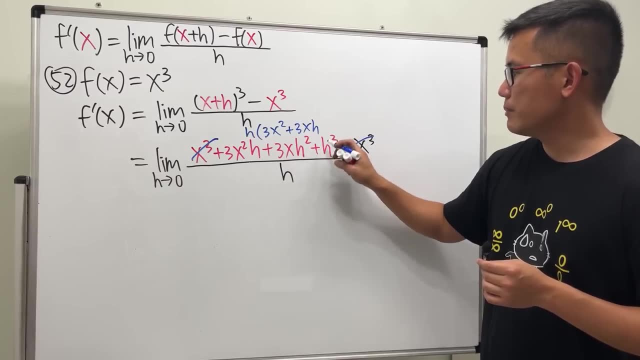 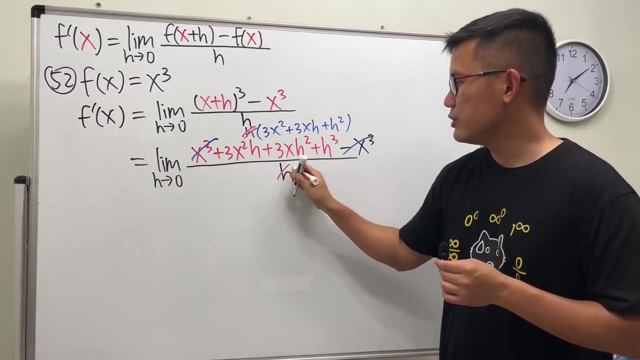 But the good thing is that we have h. We can factor that out and we get 3x squared plus 3x h and then plus h squared, And then you see that this h and that h cancel. Finally, put the 0 into this h and that h. 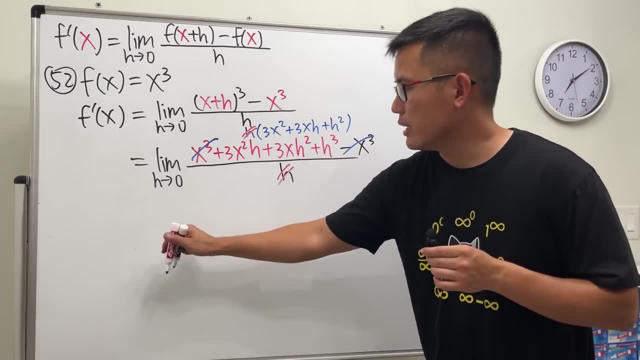 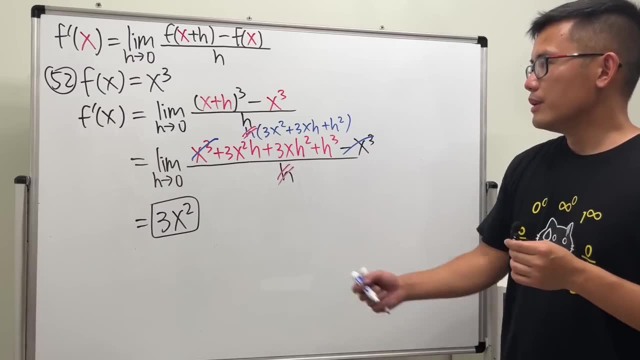 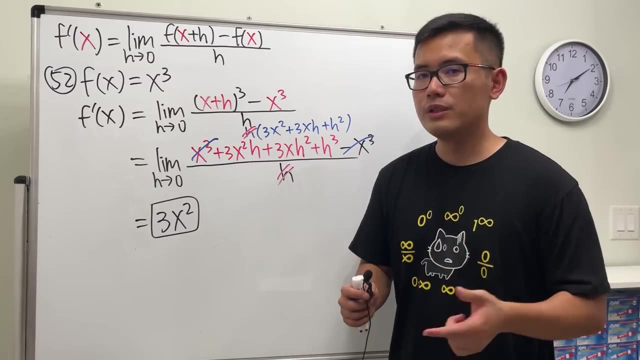 so they are gone And we get 3x squared Done. Yeah, So pretty much. if you do this, if the question is asking you the definition of derivative for extra third power, if you do this, then you will get full credit. 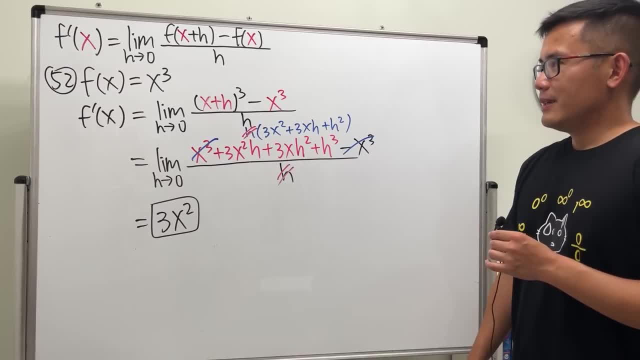 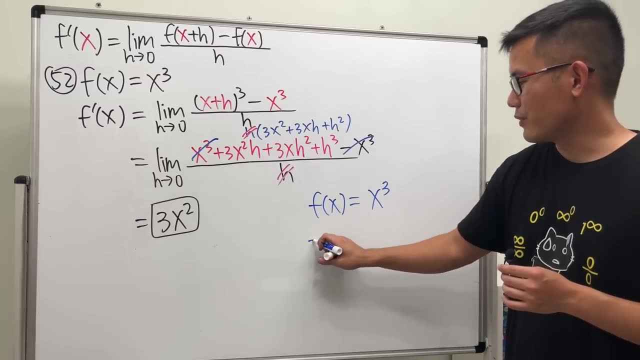 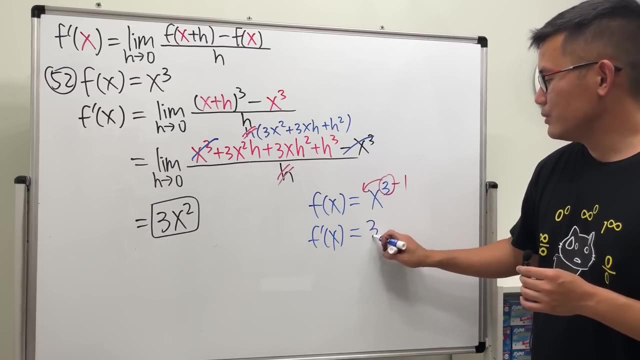 And you will be happy. You know you can, Yeah, But you can of course check the answer in your head or so, But just don't let your professor, your teacher, your TA see it. 2 seconds, 1,, 2,, 3x squared. 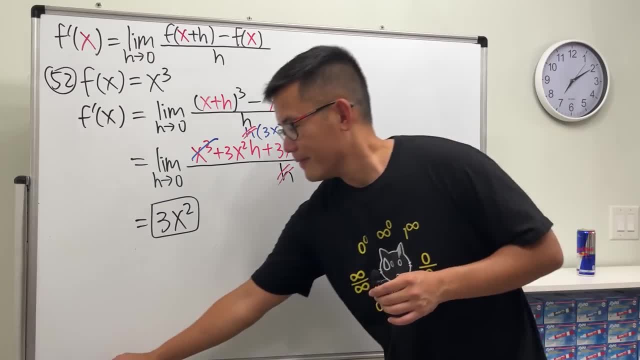 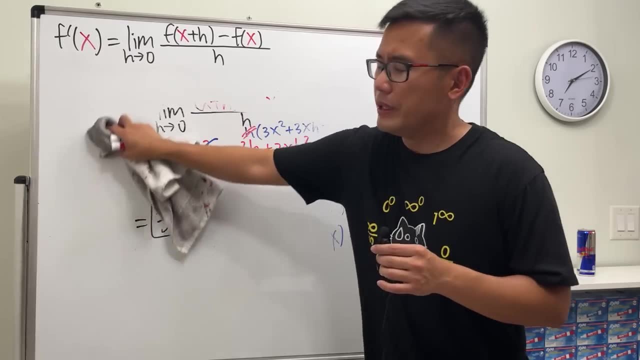 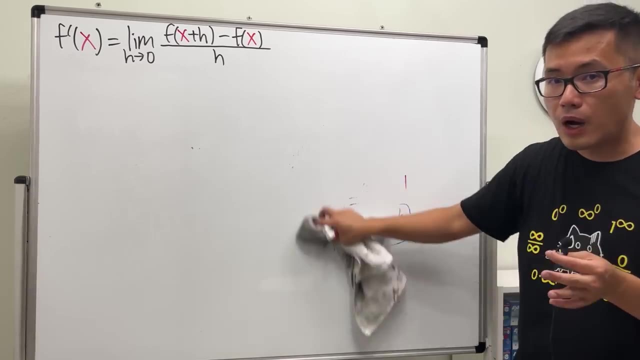 Done, Yeah, Okay. So now let's see. We have the power rule already. Why do we need the definition of derivative right? Well, of course, The reason is because the power rule only works for x to some power, x to some power. 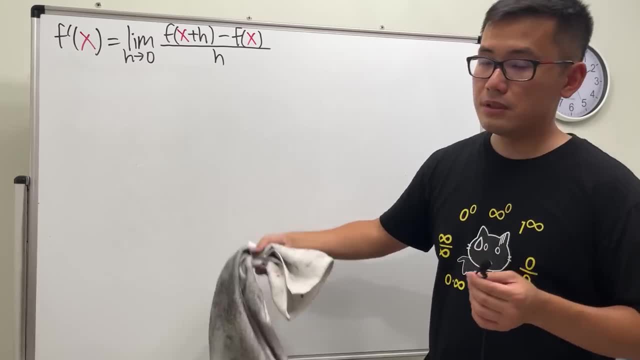 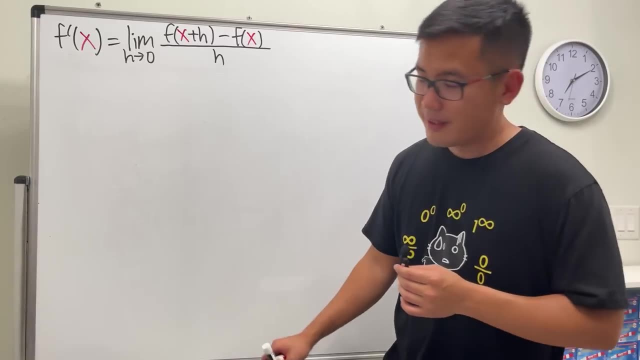 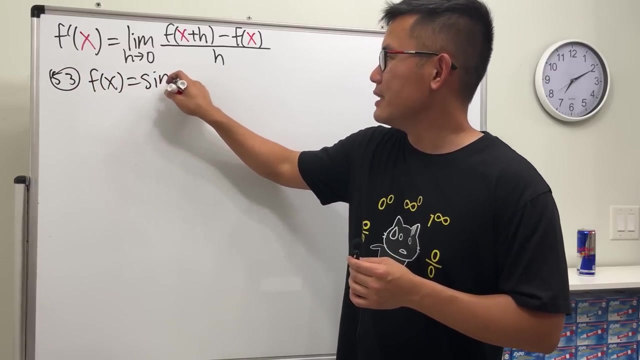 If we don't have x to some power, then oops, Uh, oh Yeah, I don't know what other sound effect I can give you, But anyway, let's look at number 53.. f of x equals sine x. How do we do the power rule? huh. 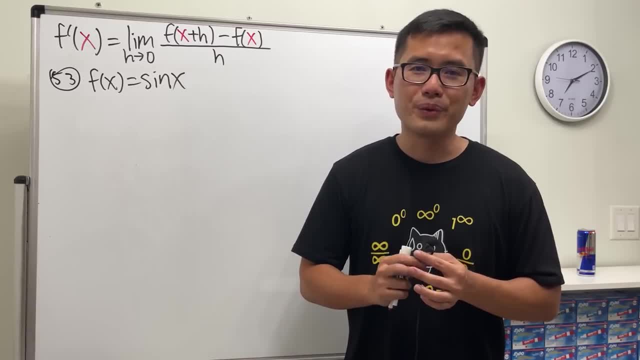 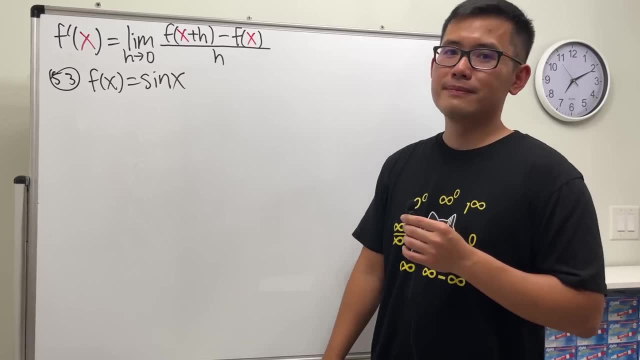 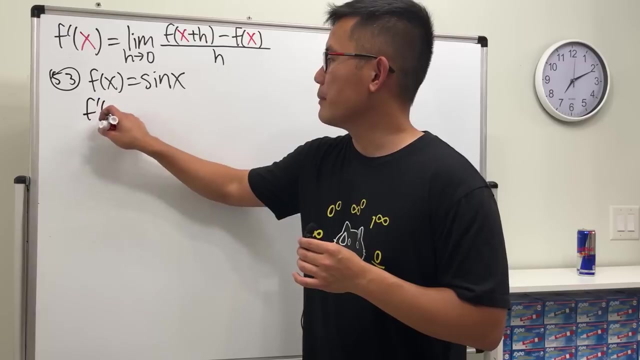 Technically you can still do the power rule, But you will have to take calculus 2. Because you have to write this as a power series and use the power rule. But let's not go there yet, Anyway. f- prime of x. 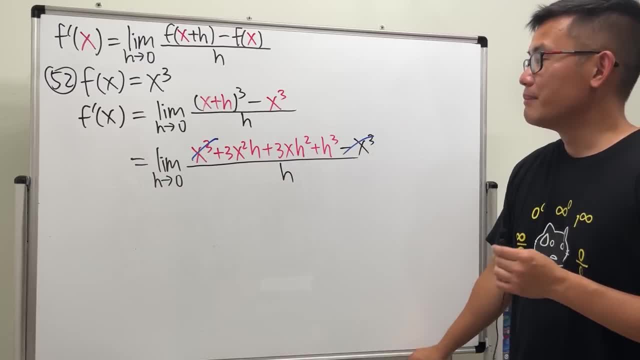 minus x to the third power o of h, minus x to the third power o of h. we can only cancel one thing. we can only cancel one thing. we can only cancel one thing. but the good thing is that. but the good thing is that. but the good thing is that you have h. you can factor that out and 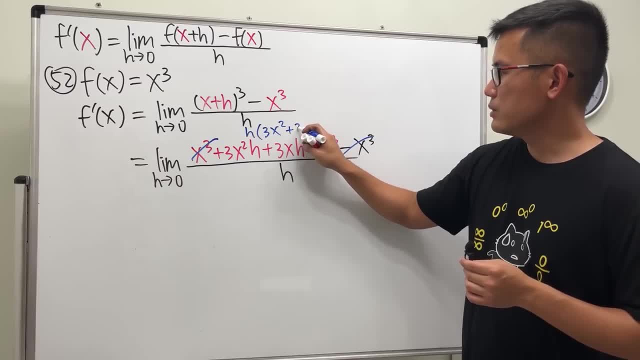 you have h, you can factor that out. and you have h, you can factor that out, and we get, we get. we get 3x squared plus 3x, 3x squared plus 3x, 3x squared plus 3x h, and then plus h squared. 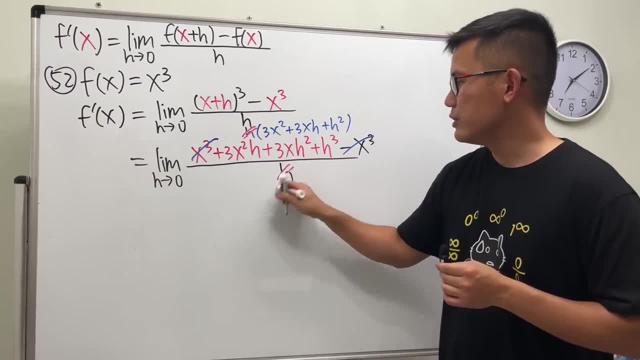 h and then plus h- squared h, and then plus h- squared okay. and then you see that this h and okay, and then you see that this h and okay. and then you see that this h and that h cancel, that h cancel, that h cancel. finally, put the zero into this h and 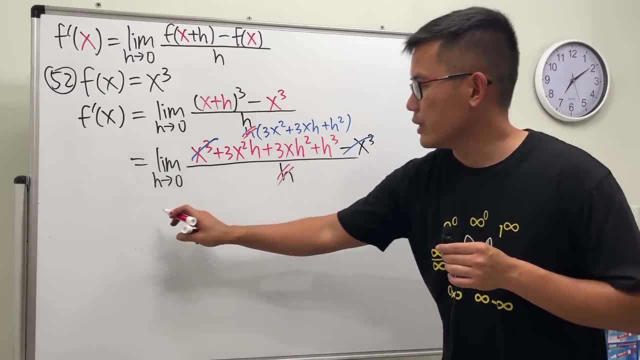 finally put the zero into this h and finally put the zero into this h and that h, so that h, so that h. so they are gone and we get 3x squared. they are gone and we get 3x squared. they are gone and we get 3x squared done. 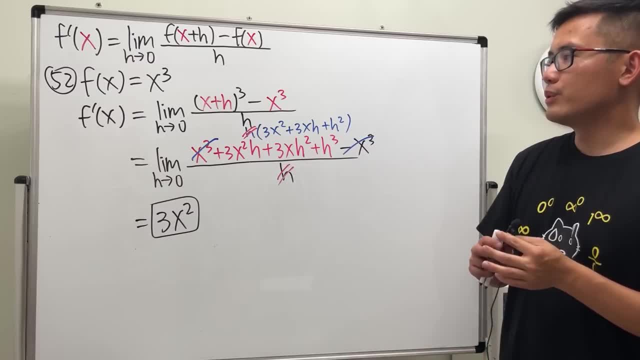 done, done, yeah, yeah, yeah, so pretty much if you do this, if the so pretty much if you do this, if the so pretty much if you do this, if the question is asking you question is asking you question, is asking you the definition of derivative for extra. the definition of derivative for extra. 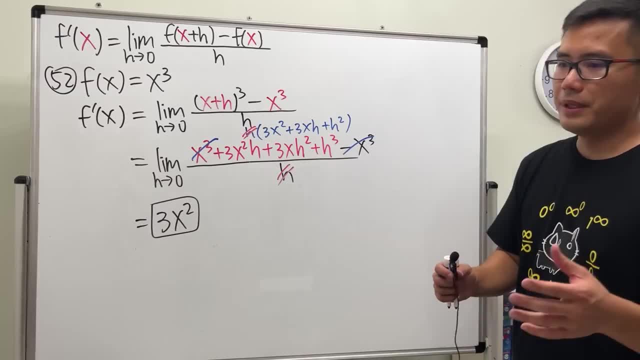 the definition of derivative for extra third power. if you do this third power, if you do this third power, if you do this, then you get full credit and you'll be. then you get full credit and you'll be. then you get full credit and you'll be happy. 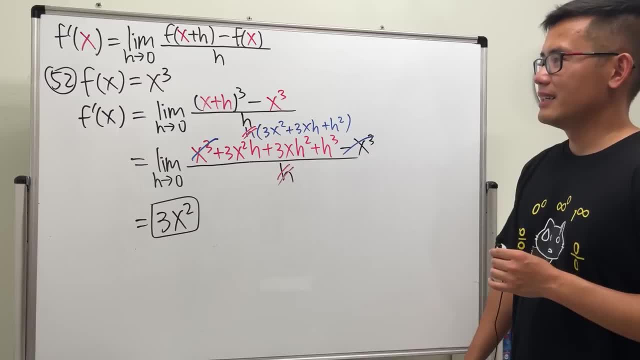 happy, happy. you know, you can, you know, you can, you know you can. yeah, yeah, yeah, but you can of course check the answer. but you can of course check the answer, but you can of course check the answer in your head, or so, in your head, or so. 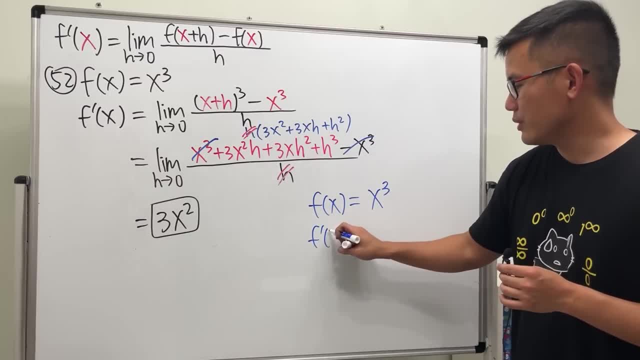 in your head or so. but just don't let your professor your, but just don't let your professor your, but just don't let your professor, your teacher, your teacher, your teacher, your tac is, tac, is tac is two seconds, two seconds, two seconds. one one, one, two. 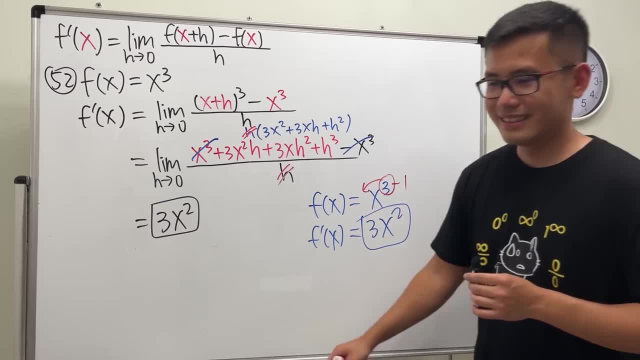 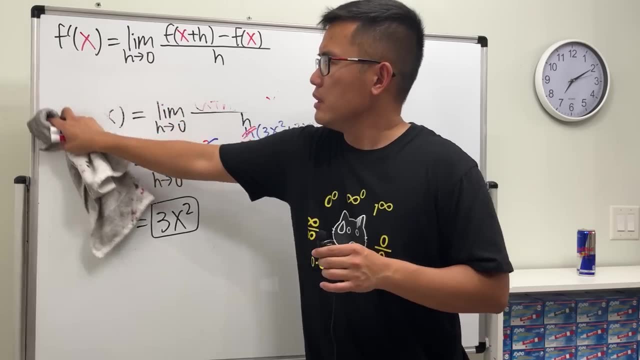 two, two, three x squared done, three x squared done, three x squared done. yeah, yeah, yeah, okay, okay, okay, so now, so now, so now let's see, let's see, let's see, we have the power rule already. we have the power rule already. we have the power rule already. why do we need the definition of? 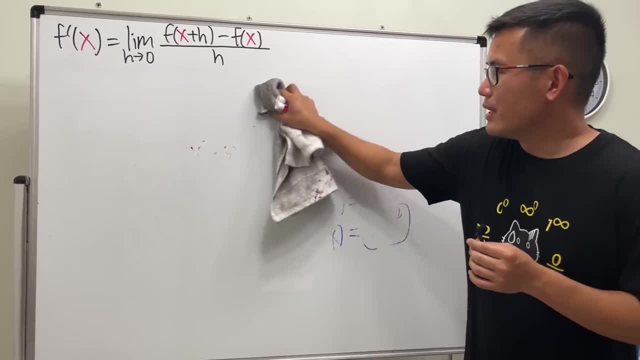 why do we need the definition of, why do we need the definition of derivative right? derivative right, derivative right: well, of course, well, of course, well, of course. the reason is because the power rule. the reason is because the power rule, the reason is because the power rule only works for x, to some power. 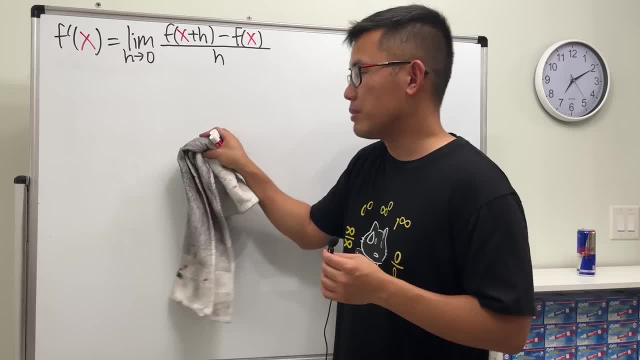 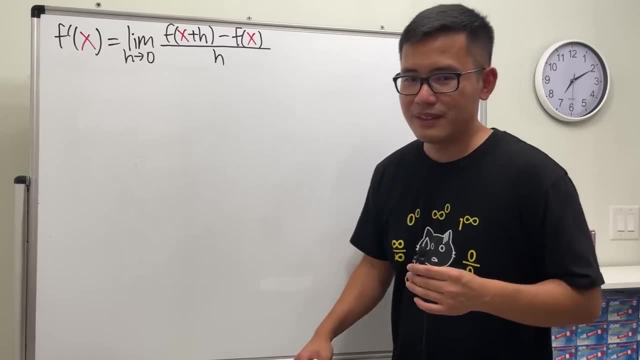 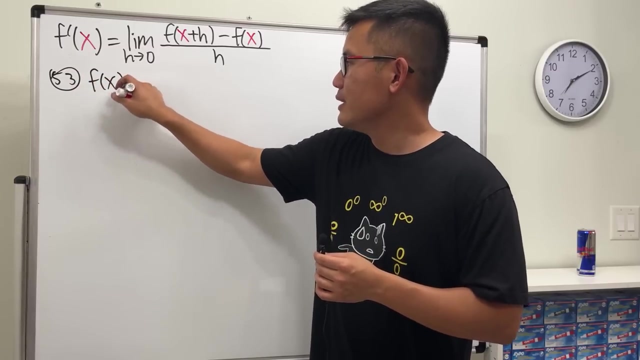 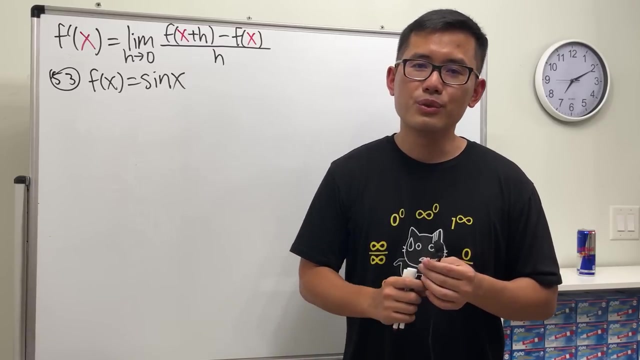 only works for x to some power, right x to some power. if we don't have x to some power, then oops, oh, oh yeah, i don't know what other sound effect i can give you. but anyway, let's look at number 53. f of x equals sine x. how do we do the power rule? technically you can still do the power rule, but 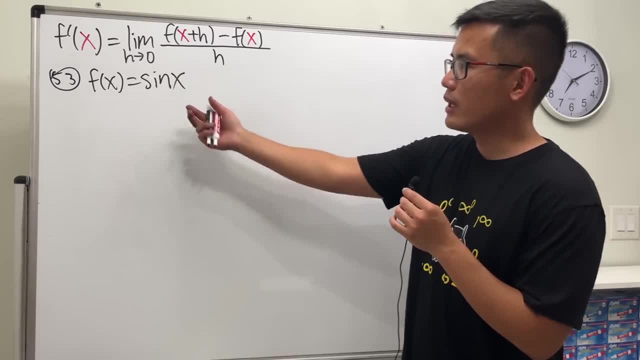 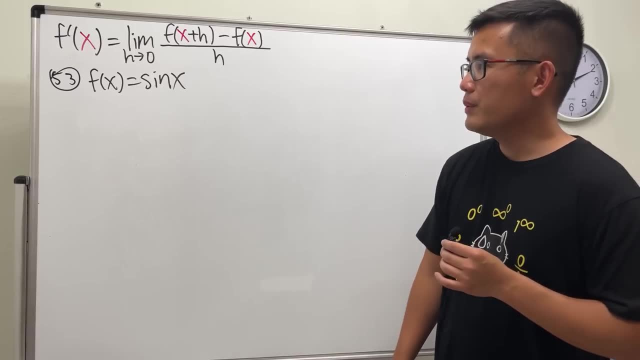 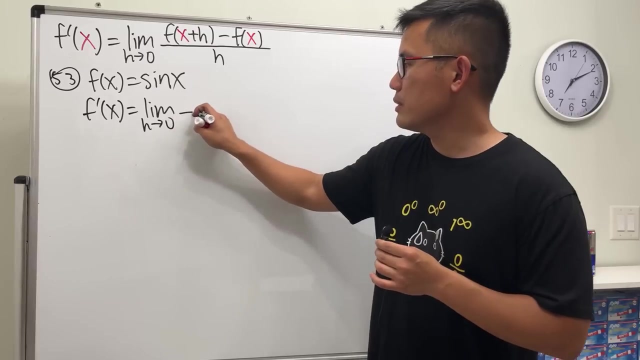 you will have to take calculus 2 because you have to write this as a power series and use the power rule. but let's not go there yet anyway. f- prime of x, limit as h approaching zero. right, if we cannot use the power rule, use the definition of derivative. 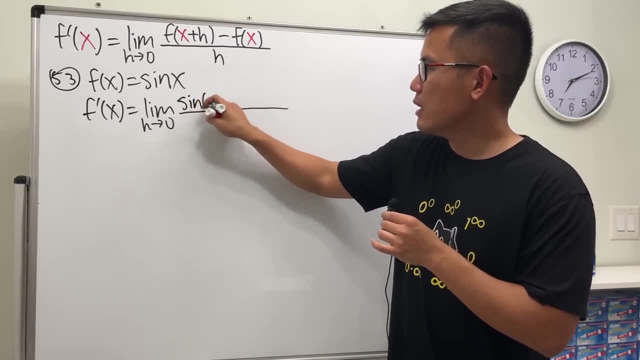 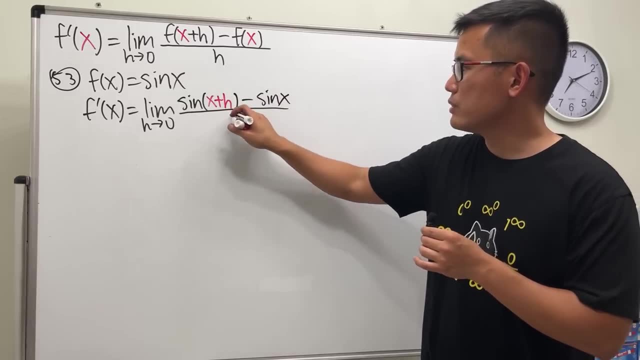 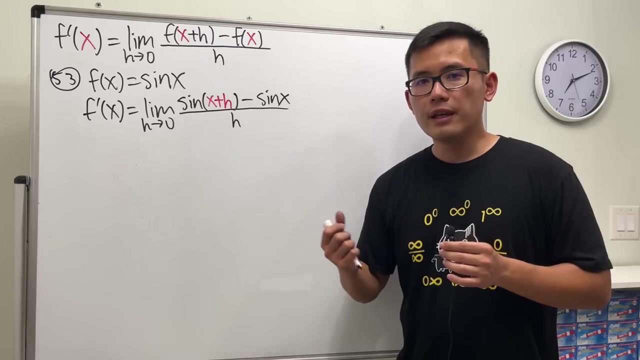 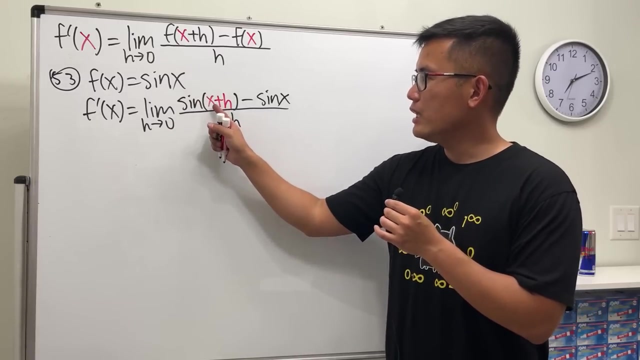 firstly, put the x plus h into here, so we have sine of x plus h and then minus the origin, not just x, and then over h. well, as i told you, whenever we use this definition, we will think about how to expand it, especially the bigger part, which is this: and we do have a way to expand this. this is just a angle. some 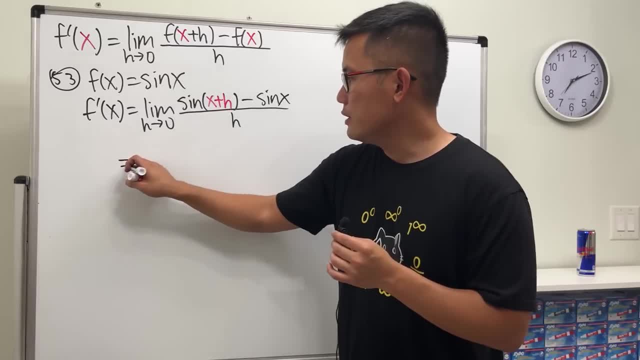 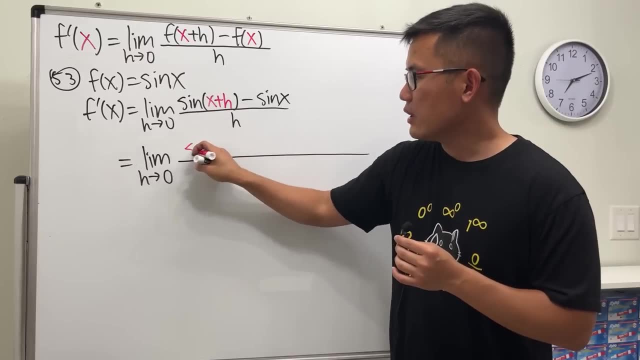 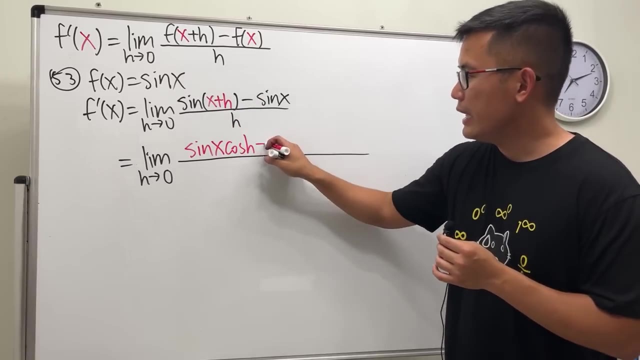 formula for sine, and i'll tell you, guess what the formula is. this right here: still limit as h approaching zero, we will first get sine of the first thing, which is x times cosine of the second, which is h, and then we add sine of the second, so sine of h times cosine. 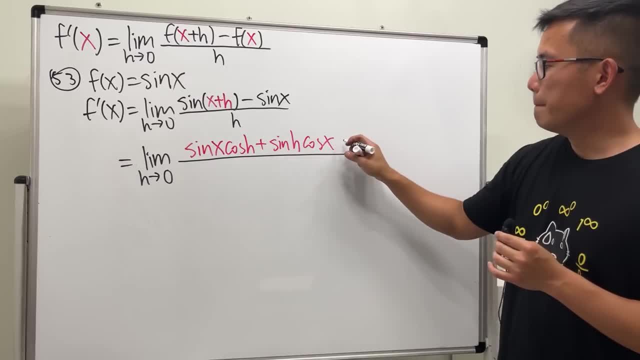 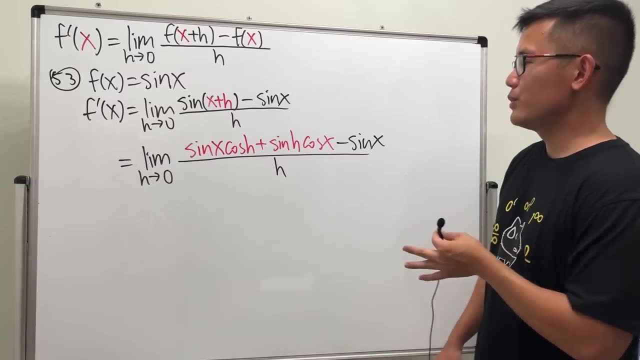 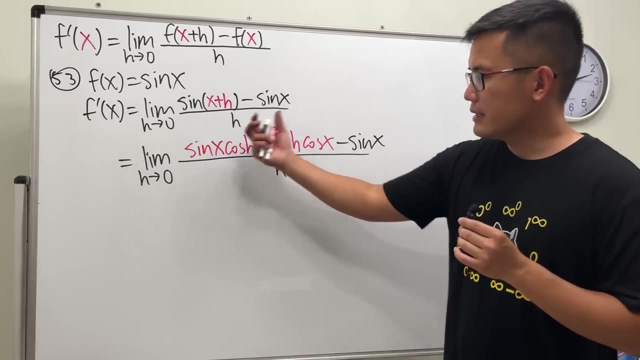 of the first. so inside this, and then minus sine of x and over h, cool, impressive. but what do you do next? well, keep this in mind. this is the limit as h approaching zero. so this is like in the h world, that if you don't have h, like for example the sine x, you can actually put it on the outside. 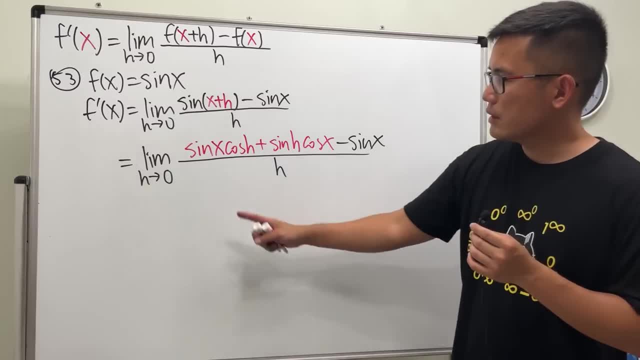 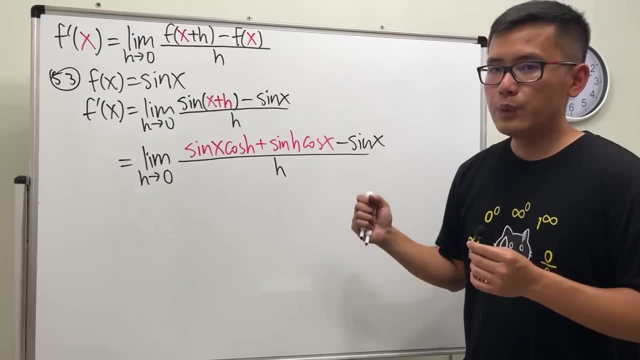 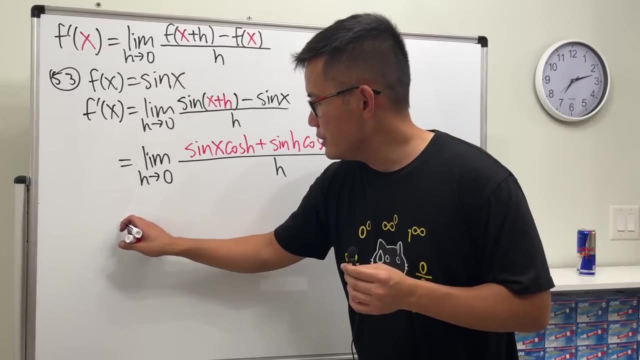 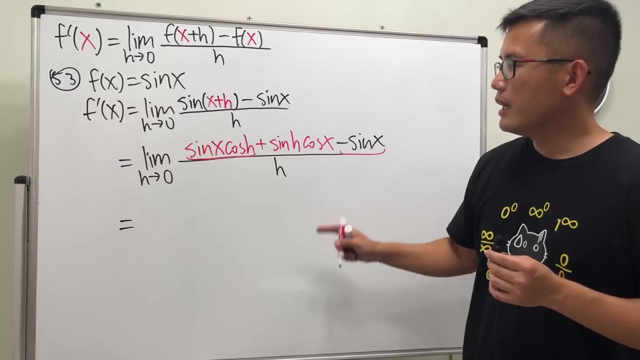 of the limit and don't worry about it. so have a look, this term has sine x, this term also have the sine x. we can put them together and we can factor out the sine x and then kick it outside of the limit. so let's do two things right now. i'm going to pair this and that right here, okay, and then 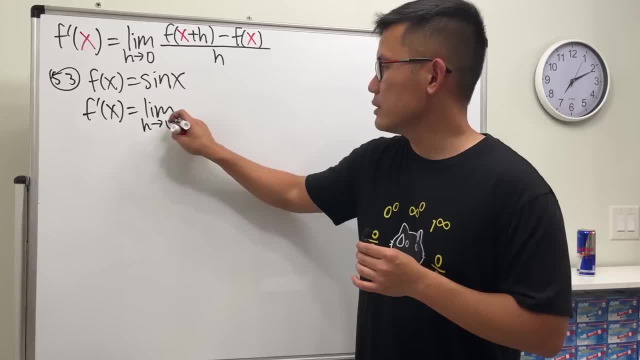 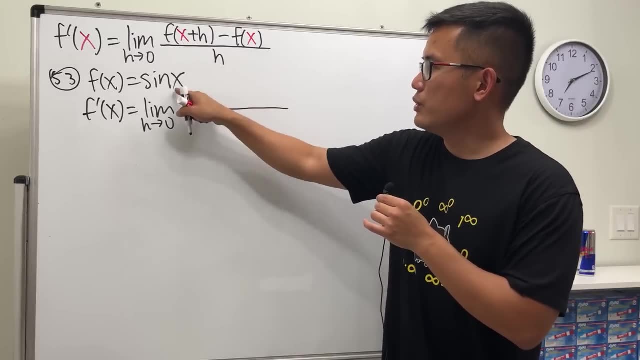 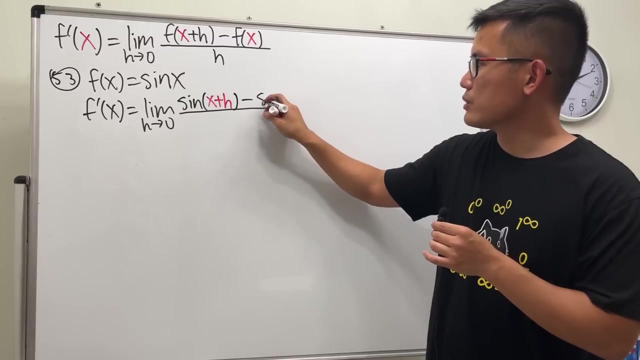 limit as h approaching 0. Right, If we cannot use the power rule, use the definition of derivative. Firstly, put the x plus h into here, So we have sine of x plus h And then minus the original, just sine x. 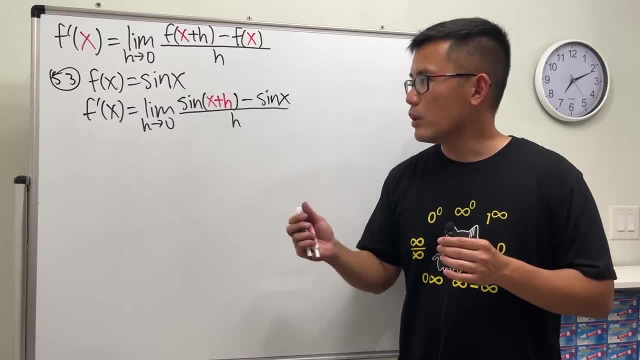 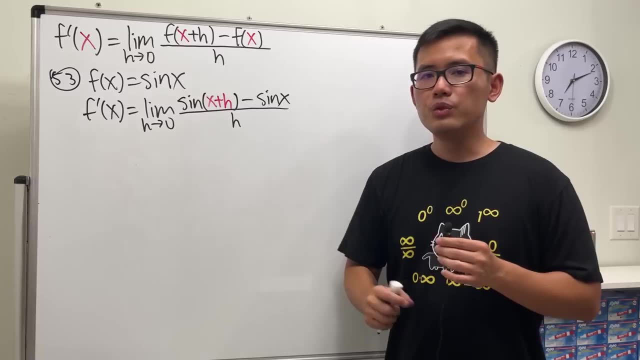 And then over h. Well, as I told you, whenever we use this definition, we will think about how to expand it, Especially the bigger part, which is this: And we do have a way to expand this. This is just a formula for sine. 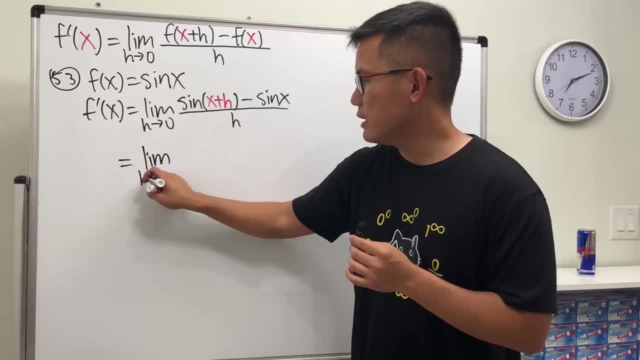 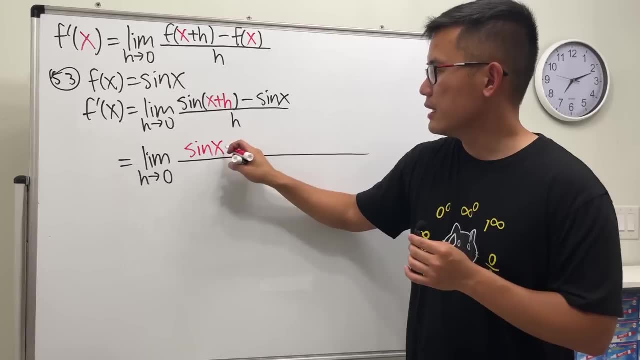 And I'll tell you guys what the formula is This right here: still limit as h approaching 0.. We will first get sine of the first thing, which is x, times cosine of the second, which is h, And then we add: 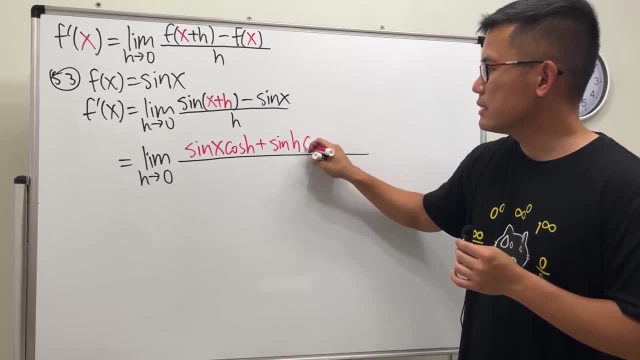 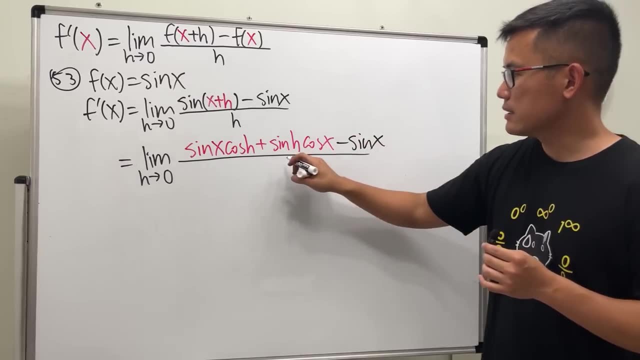 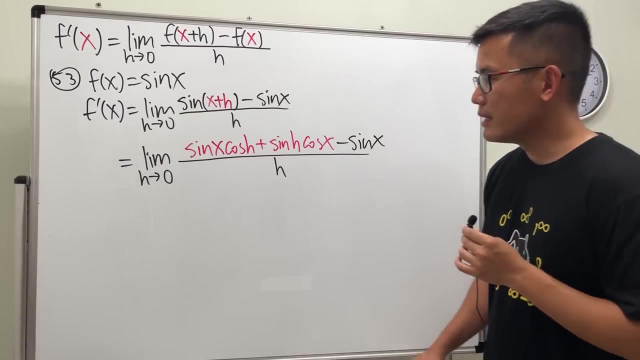 sine of the second, so sine of h times cosine of the first. So it's like this: And then minus sine of x and over h. Cool, Impressive. but what do we do next? Well, keep this in mind. 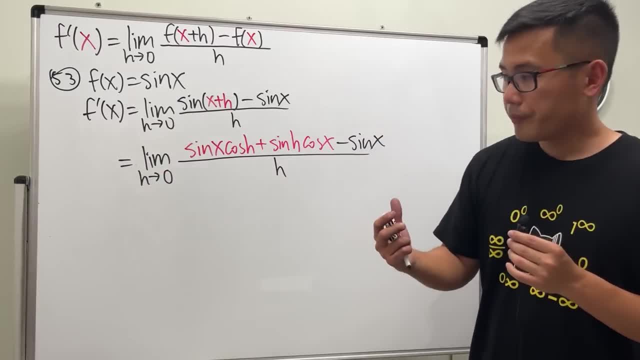 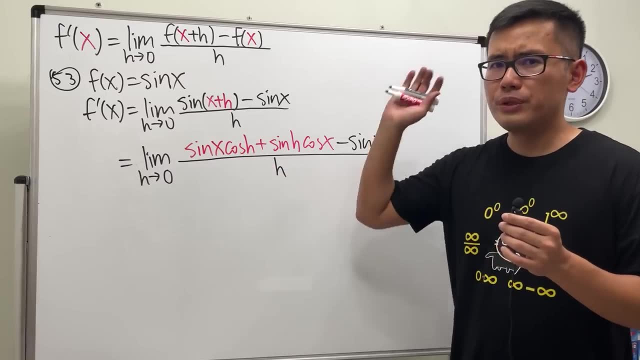 This is the limit as h approaching 0. So this is like in the h world, Meaning that if you don't have h, like for example the sine x, you can actually put it on the outside of the limit And don't worry about it. 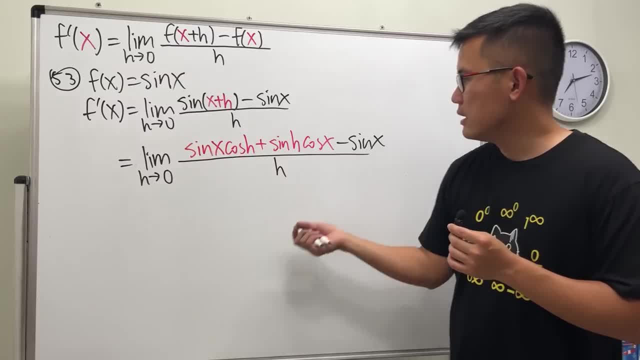 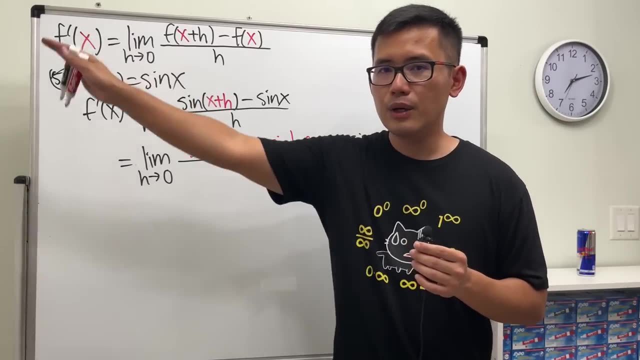 So have a look, This term has sine x, This term also has the sine x. We can put them together and we can factor out the sine x And then kick it outside of the limit. So let's do two things right now. 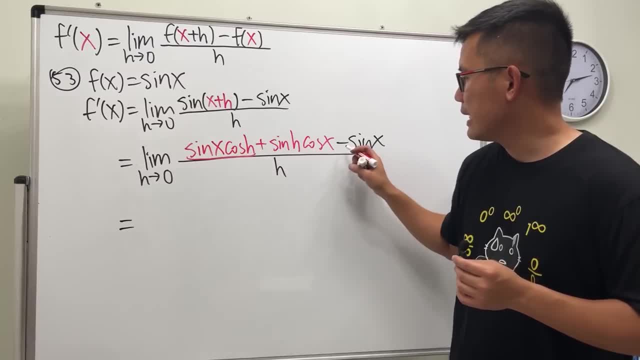 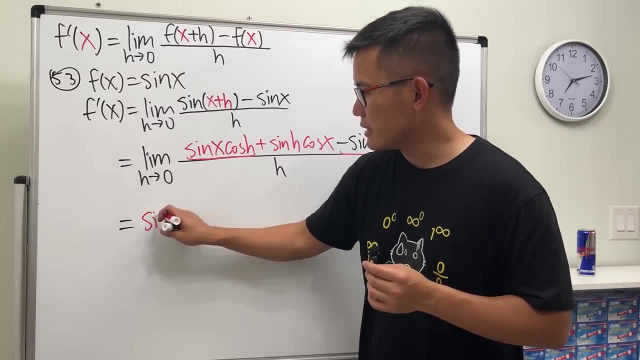 I'm going to pair this and that right here, okay, And then I'll factor out the sine x and then put it on the outside of the limit. So we have the sine x right here, and then let's look at the limit. 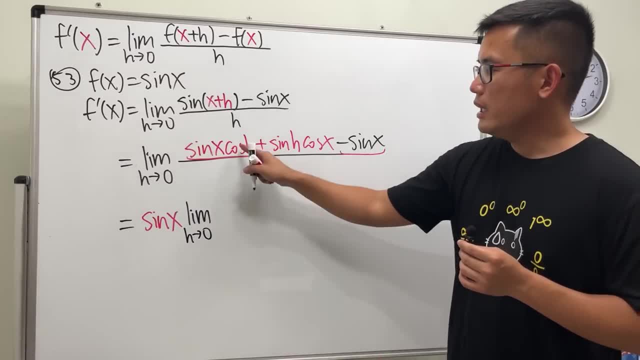 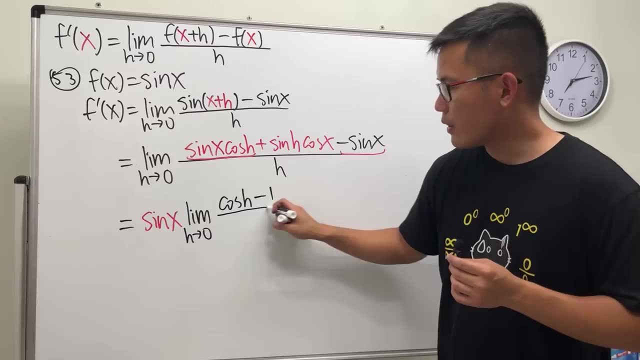 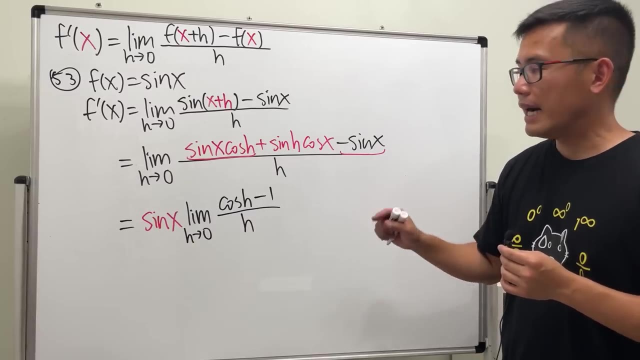 as h approaching 0. Here we'll just have cosine of h and then minus 1, and then over h We still have that denominator, Alright, And of course we have other stuff too. But for the other stuff it's this over. 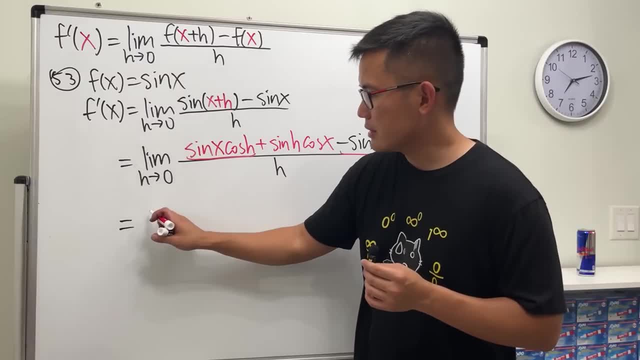 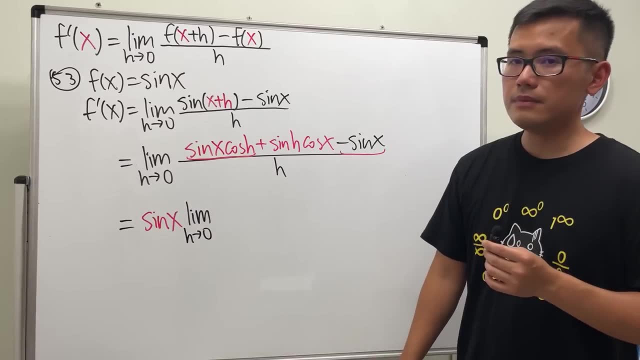 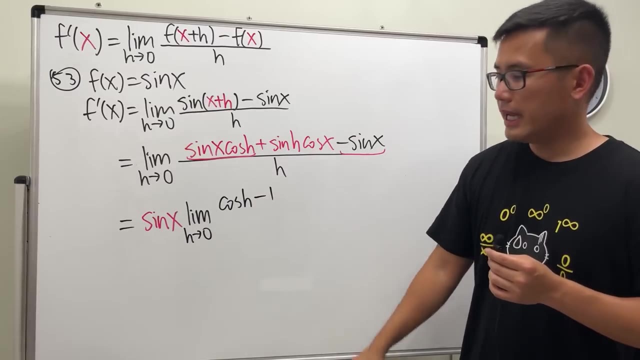 factor out the sine x and then put it on the outside of the limit. so we have the sine x right here, and then let's look at the limit as h approaching zero. here we'll just have cosine of h and then minus one, and then over h i still have that denominator. all right, and of course we 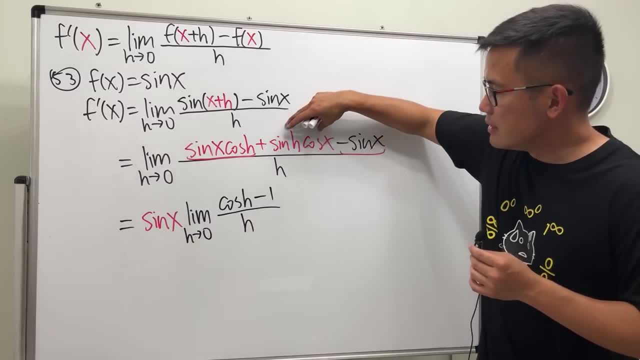 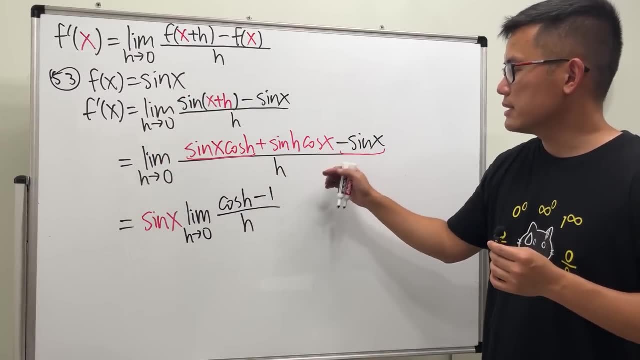 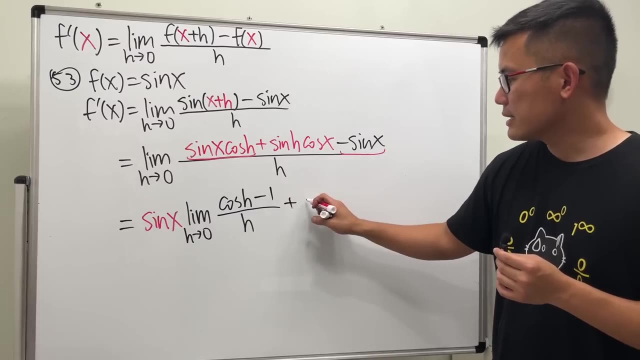 have other stuff too, but for the other stuff is this over h and then we can take the limit of that. so let's break it apart. let's also put a cosine x outside. so i'm looking at this right now for the second part, i'm going to add cosine x on the outside. same reason: because it doesn't have the 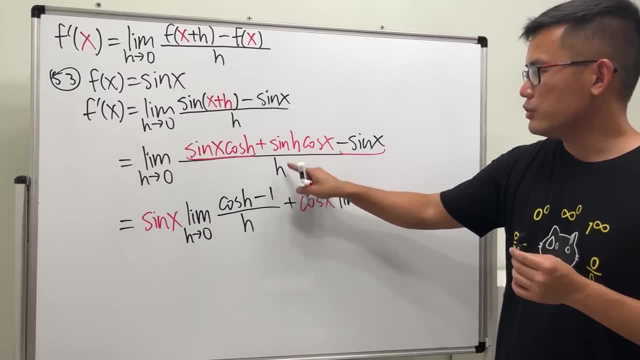 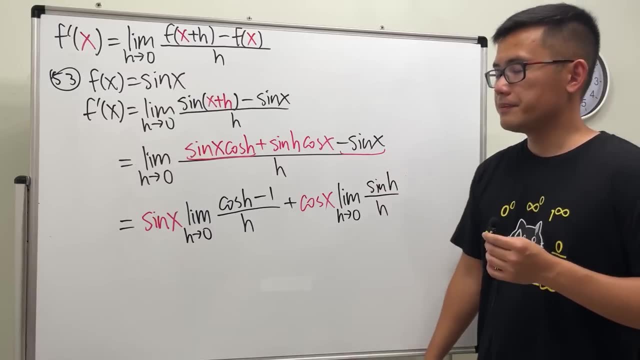 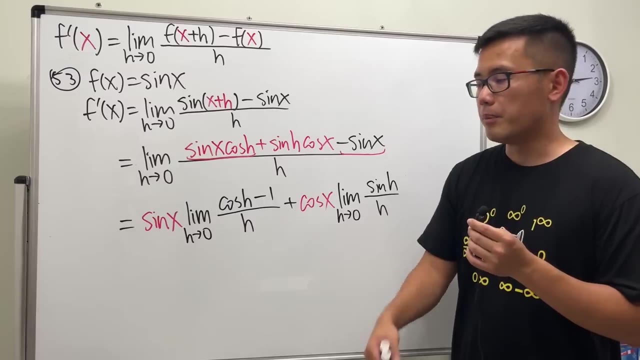 h and then we just focus on the limit of sine h over h as h approaching zero. all right. so the reason that we can do this is limit of a sum. it's the sum of the limits, so you can break them apart. and also, if you don't have the h, then you can put. 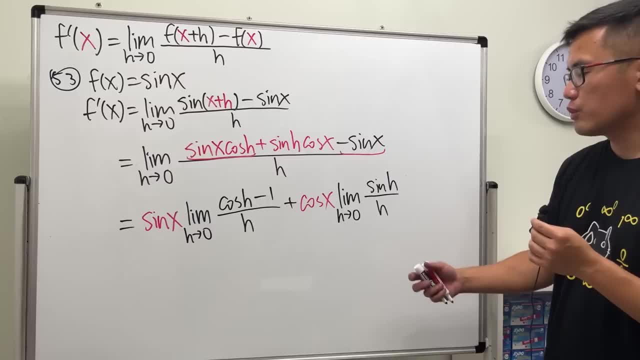 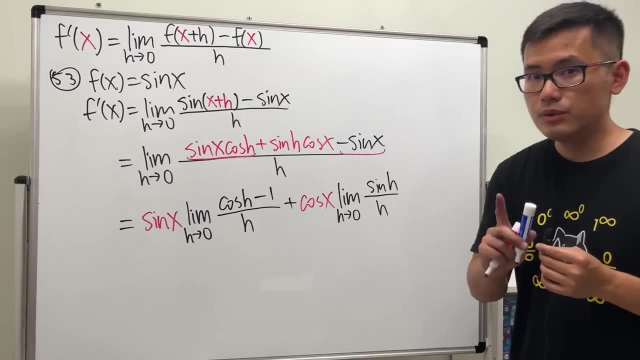 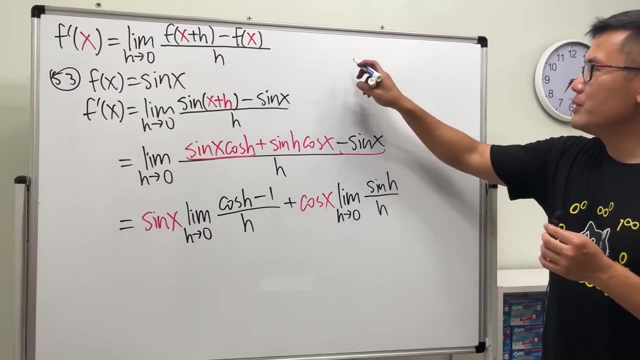 the expression on the outside of the limit. so that's why we are doing, that's why we can do this. okay, this right here, we get zero for zero. likewise that. but you know what? this right here, we have seen it. question number five. so let me just remind you guys that note. 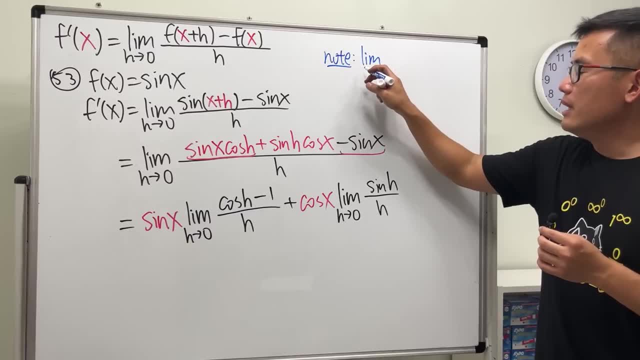 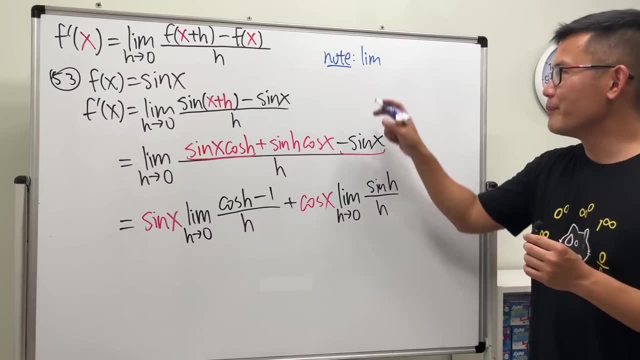 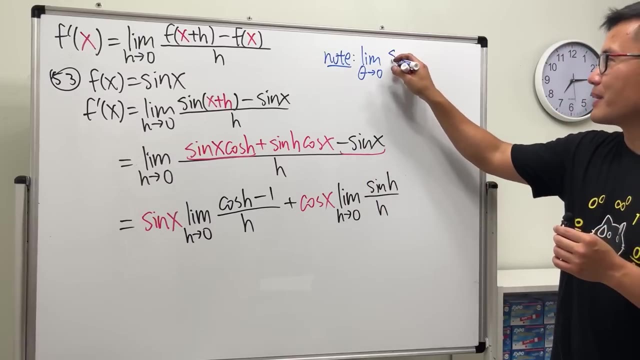 if we have the limit. i use x right now, we have h. i know i'm going to be using theta right now. i think it's like a more universal variable for this limit in particular, by the way, the sine of an angle, sine of theta over theta. this right here will give you one, and then you can see. 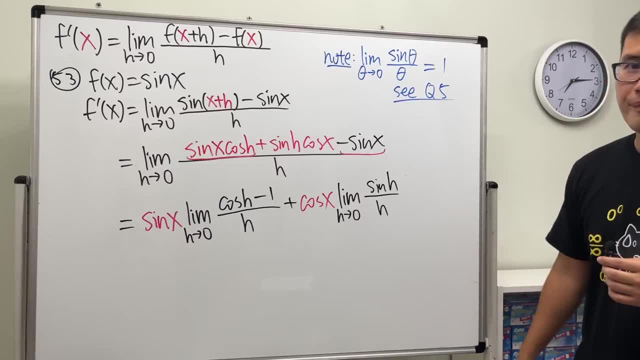 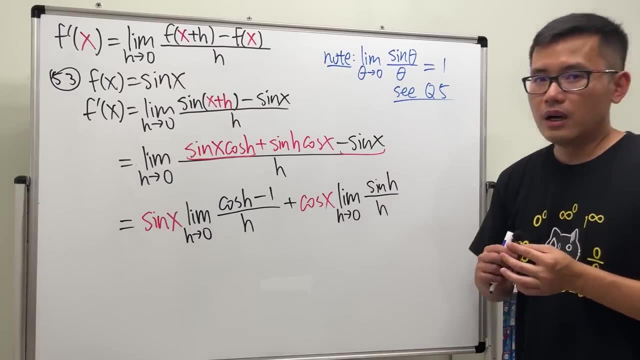 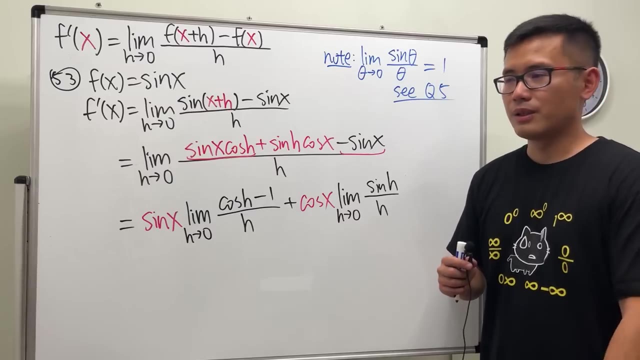 question number five: for the graph. for now, this video, i will just tell you guys, look at the graph- that we have what you can also just plug into calculator. i didn't do anything with the calculator in this video because it's just plugging the calculator right, so you should be able to just plug into. 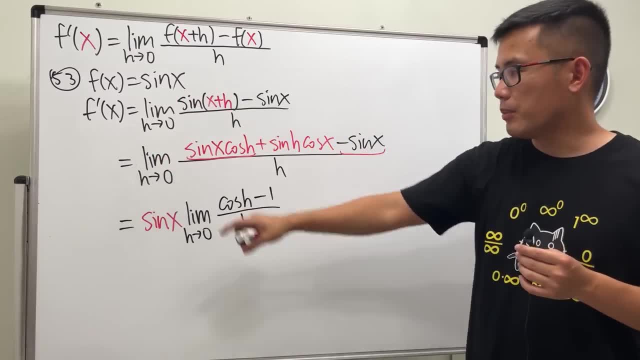 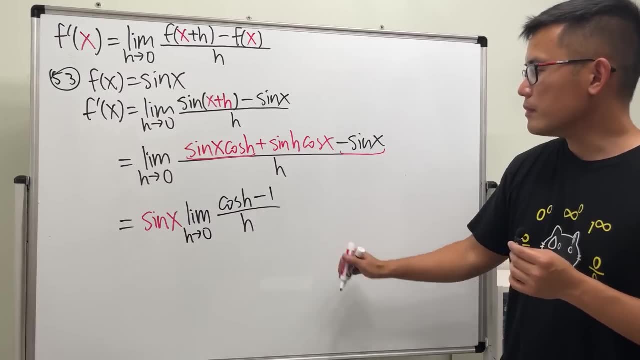 h, and then we can take the limit of that. So let's break it apart. Let's also put the cosine x outside. So I'm looking at this right now for the second part, I'm going to add cosine x on the outside. 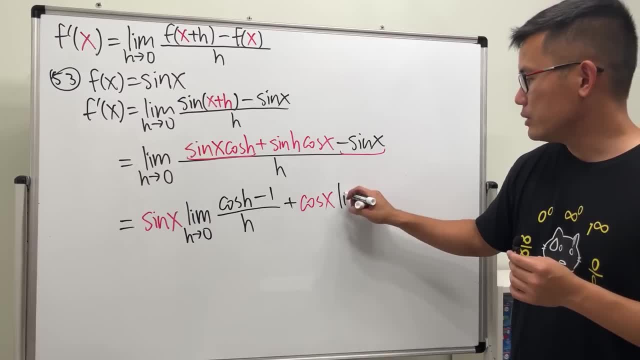 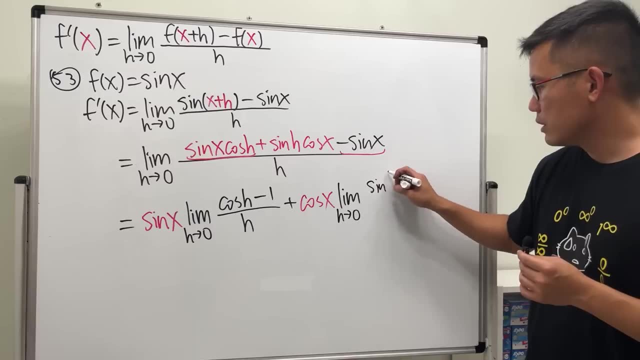 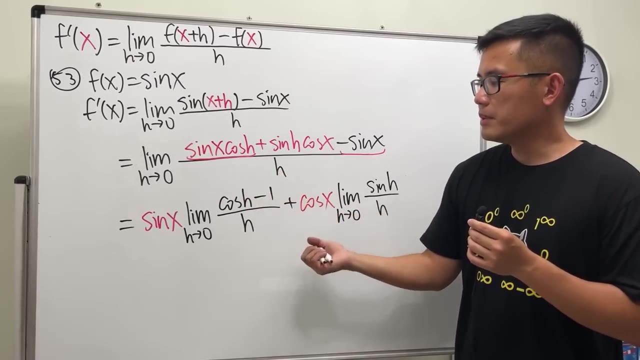 same reason, because it doesn't have the h, And then we just focus on the limit of sine h over h as h approaching 0. Alright, So the reason that we can do this is: limit over sum is the sum of the limits, so we can break them apart. 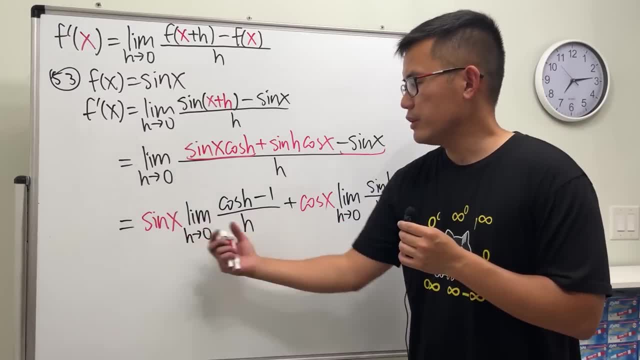 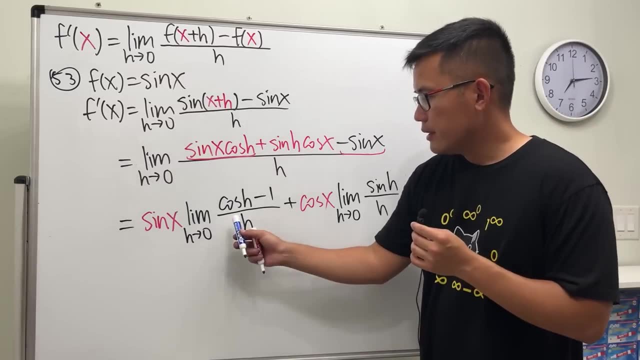 And also, if you don't have the h, then you can put the expression on the outside of the limit. So that's why we are doing, that's why we can do this. Okay, This right here: we get 0 for 0.. 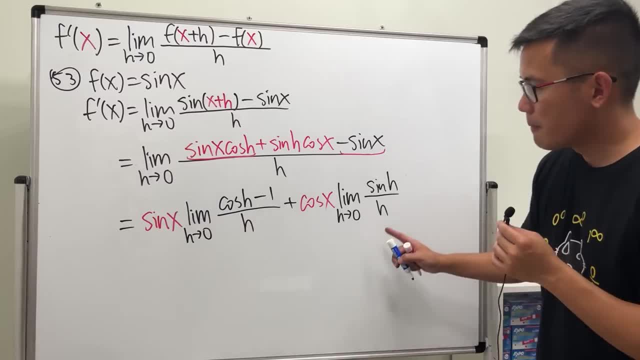 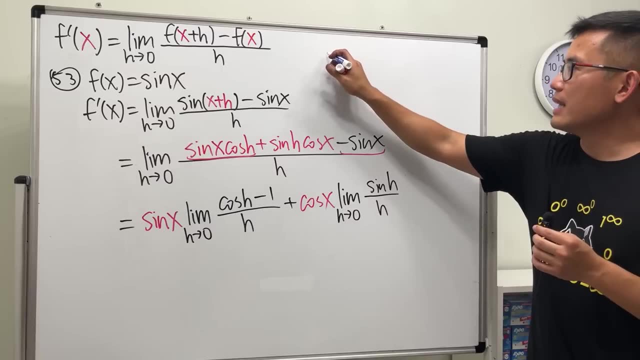 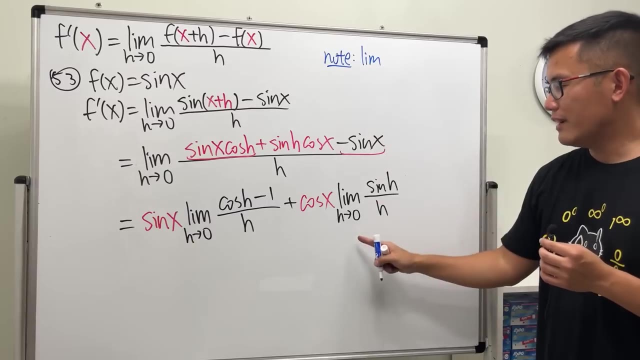 Likewise that. But you know what This? right here, we have seen it, question number 5.. So let me just remind you guys that note: if we have the limit- earlier I used x, right now we have h. 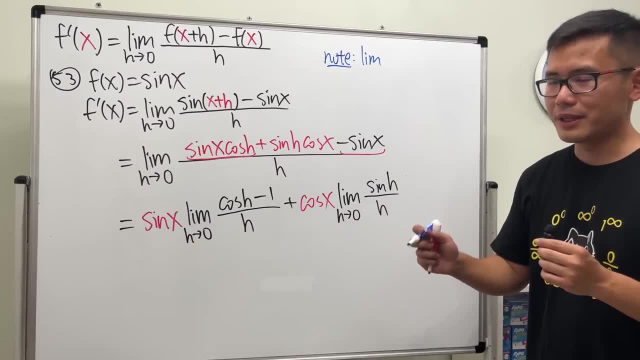 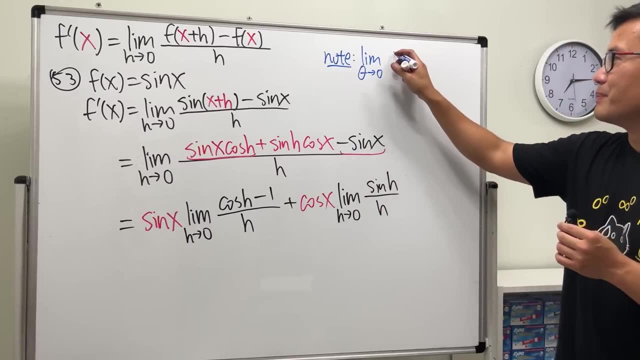 I know I'm going to be using theta right now. I think it's like a more universal variable for this limit, in particular, By the way, sine of an angle, sine of theta over theta. this right here will give you 1.. 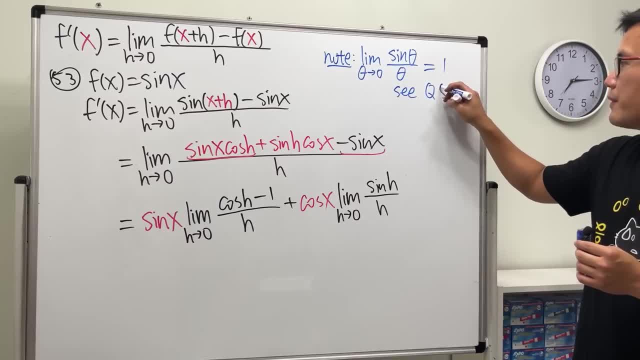 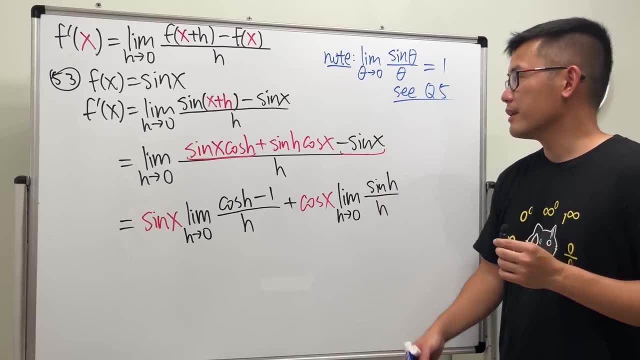 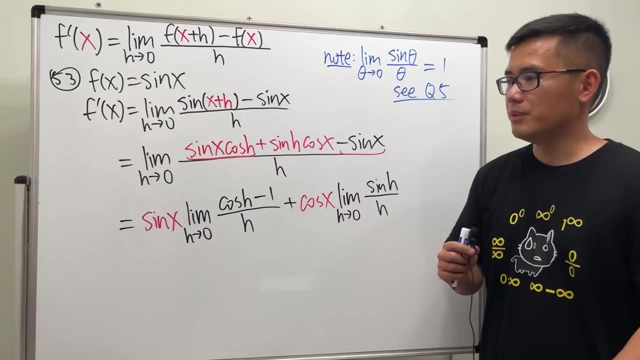 And then you can see question number 5 for the graph. For now this video. I will just take a look at the graph that we have. Well, you can also just plug in to calculator. I didn't do anything with the calculator in this video because 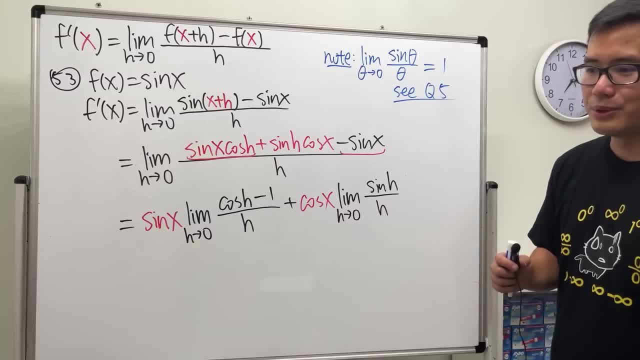 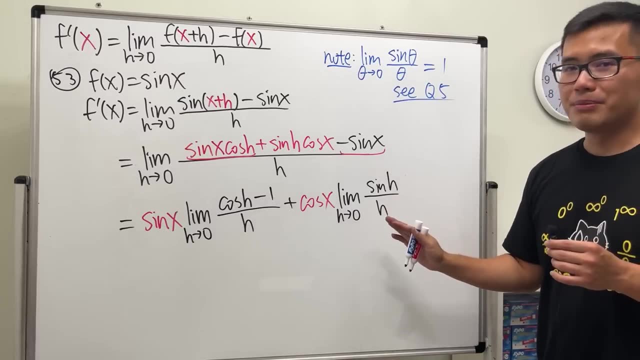 it just plug in the calculator, right? So you should be able to just plug in to the calculator. But this right here you please do not use Lapito's rule. What's Lapito's rule? Just wait for it. 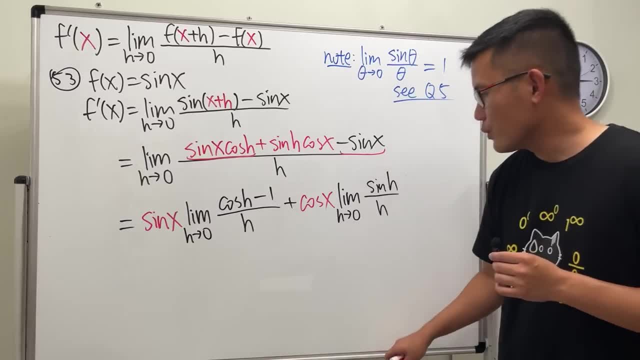 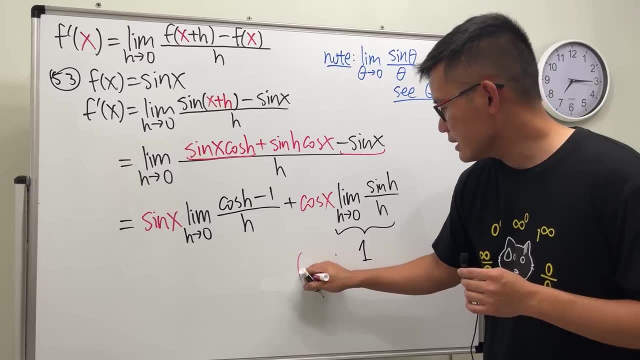 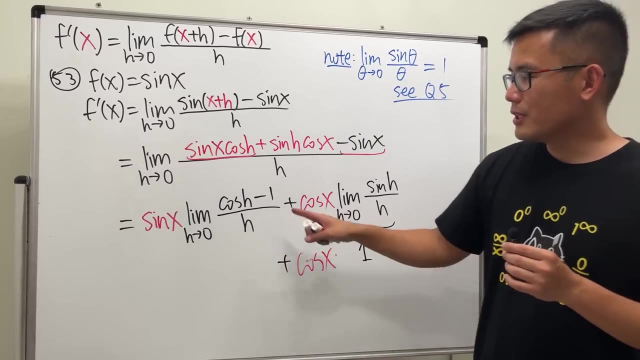 Anyway, what I'm trying to say is that this right here, per our discussion earlier, is: 1. So we have, this times cosine x, And then what's this then? In fact, you can try it: Multiply the top. 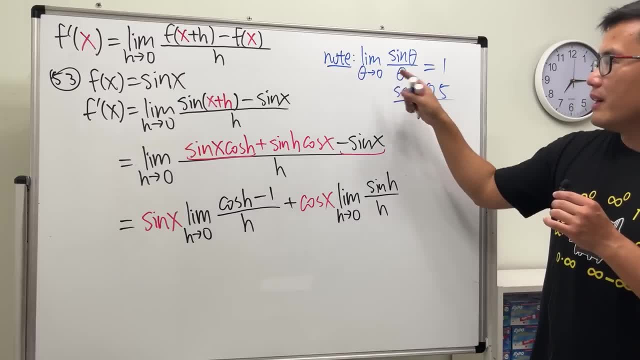 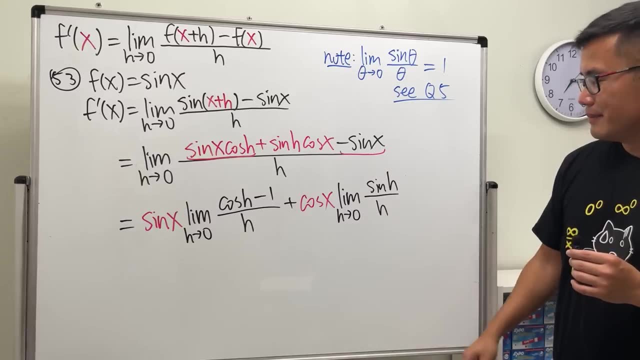 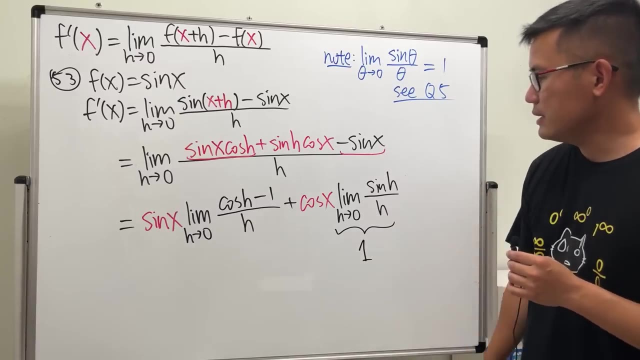 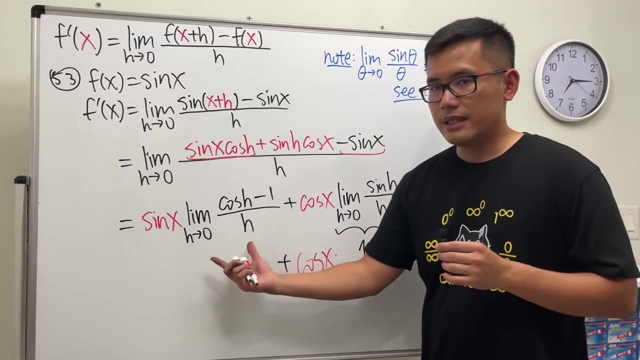 the calculator. but this right here: you please do not use lapito's rule. what's lapito's rule? just wait for it anyway, what i'm trying to say is that this right here per hour discussion earlier is one. so we have this times sin x, and then what's this? then, in fact, you can try it: multiply the top and bottom by conjugate. 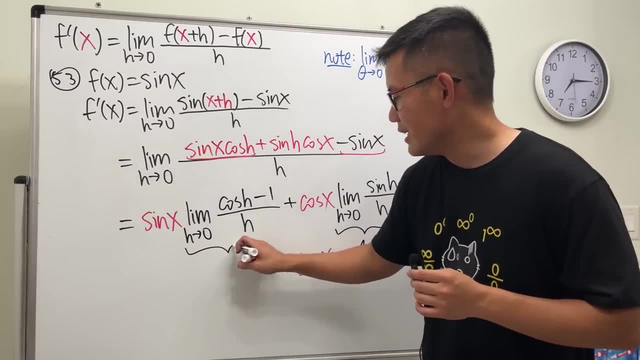 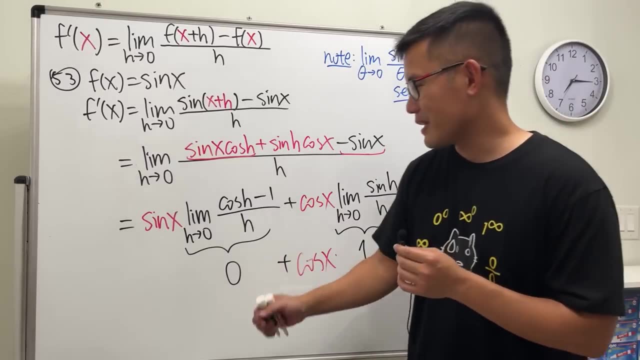 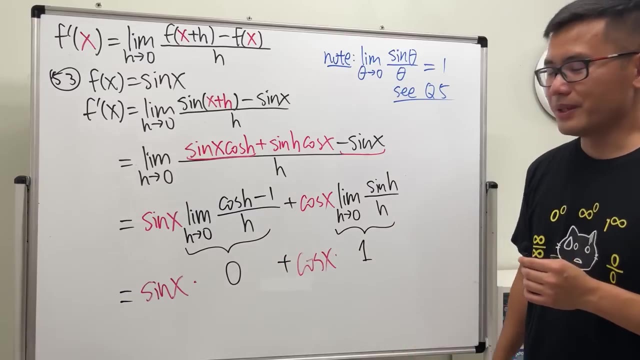 and use this to help you out. you can try it, but i will tell you the answer right here. you get zero or you can use the graph. just use a graphing calculator. use a calculator, plug in the numbers- that's not a discussion for here, but like that, that's equal to zero. so only we get what zero, cosine x? hey, the answer is: 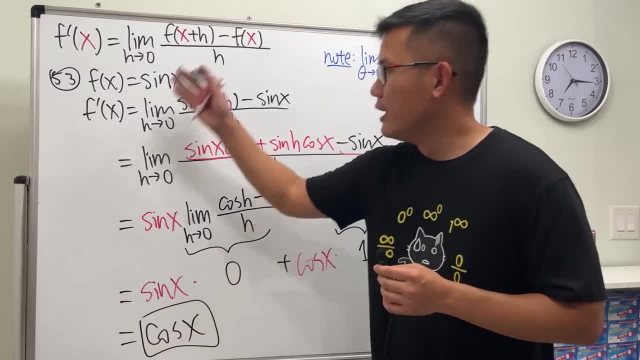 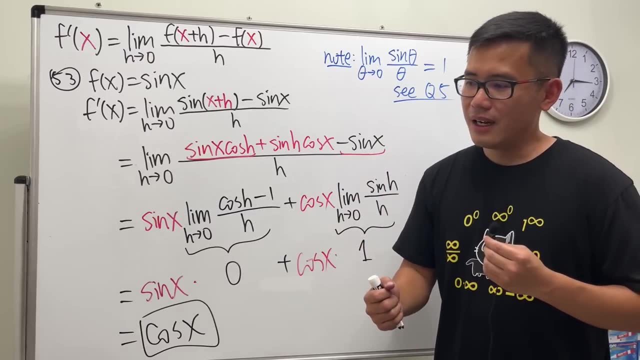 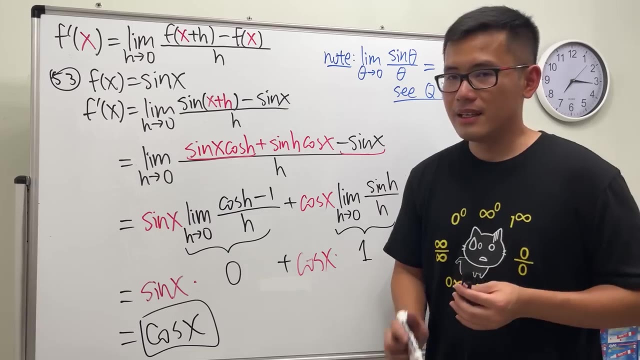 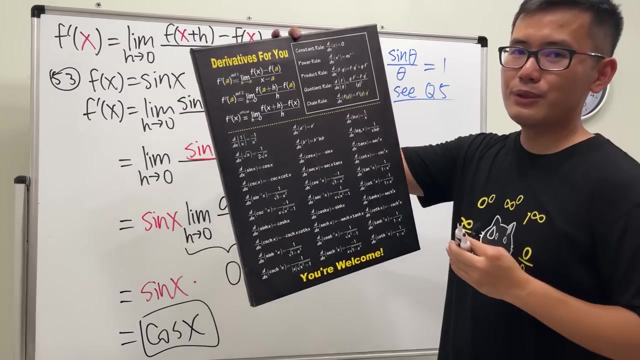 just nicely equal to cosine x. sine and cosine, yeah, they're always together in uh pre-calc trick and also calculus, of course. yeah, they don't run away from each other. yeah, and let me just make sure that i'm not missing anything here, that it is right. aha, derivative of sine x is equal to cosine x, told you. 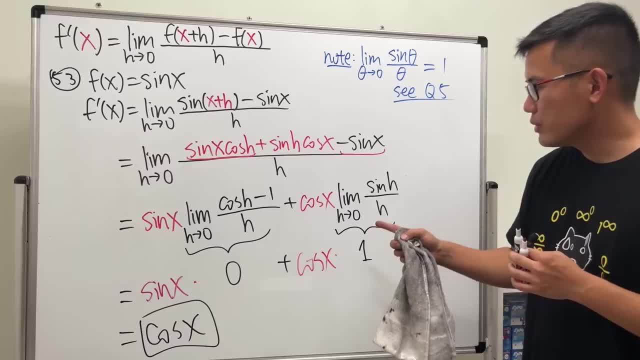 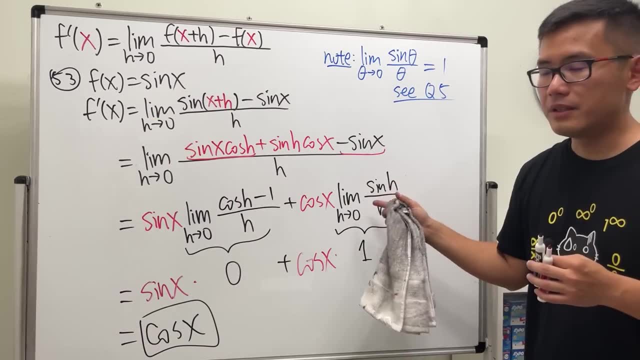 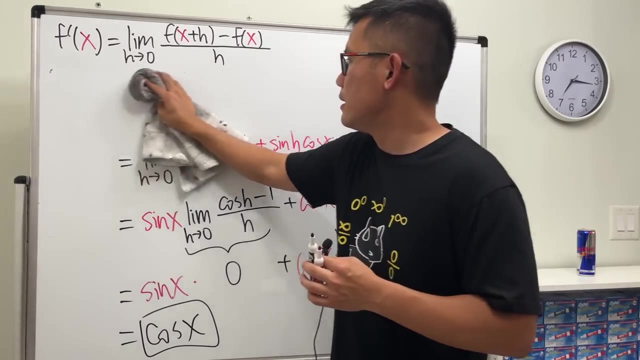 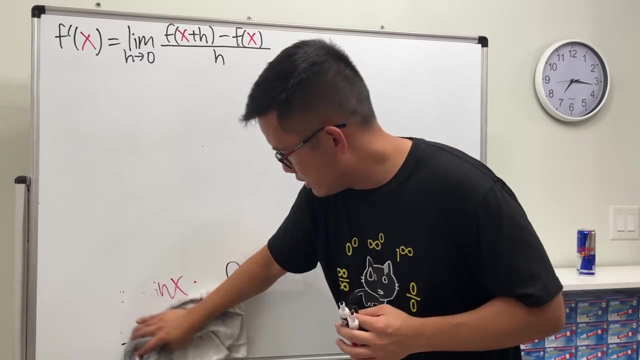 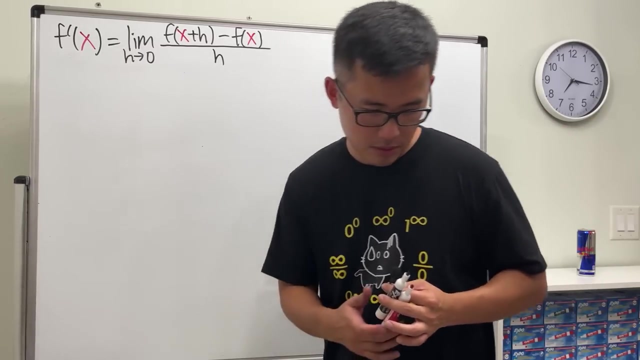 okay, anyway, i want you guys to pay attention to that. hey, we run into this limit right here when we are trying to get the derivative of sine x. this is going to show up later on, like an hour or two, i don't know, by the way. all right, so now let's take a look at 54. 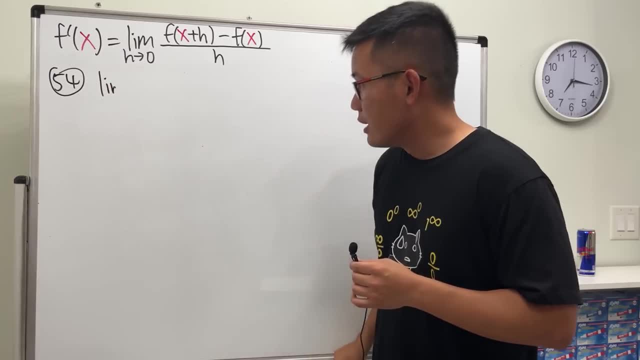 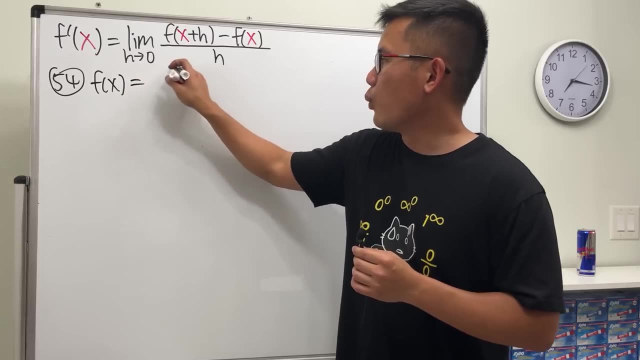 here we have the sorry- uh, we're still doing the definition of derivative number 54. we have the function f of x. this is 1 over 1 plus 8. and we have the function f of x. this is 1 over 1 plus 8. 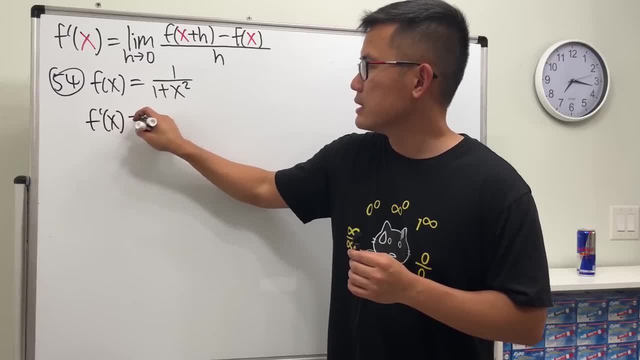 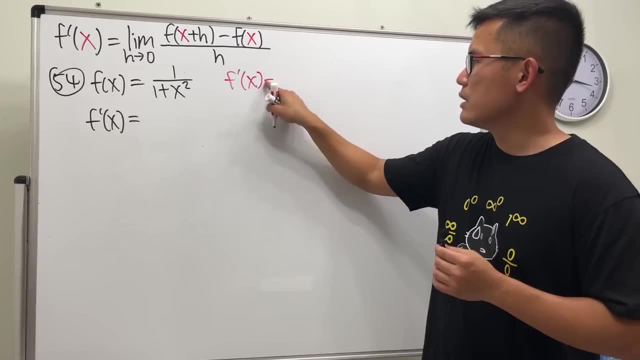 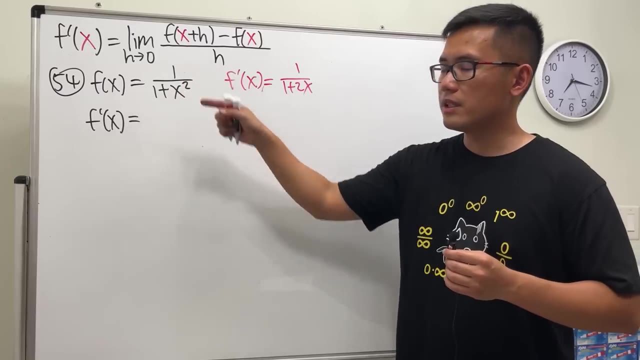 x square and then we want f prime of x. can we use the power rule right here and say the answer is f prime of x equals to the power rule, and then we get 1 over 1 plus 2x. can we put the 2 to the front minus 1? 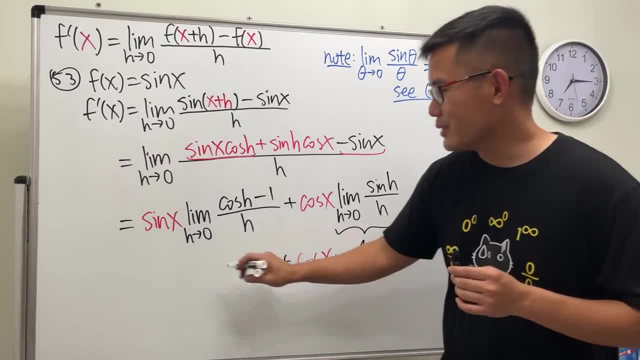 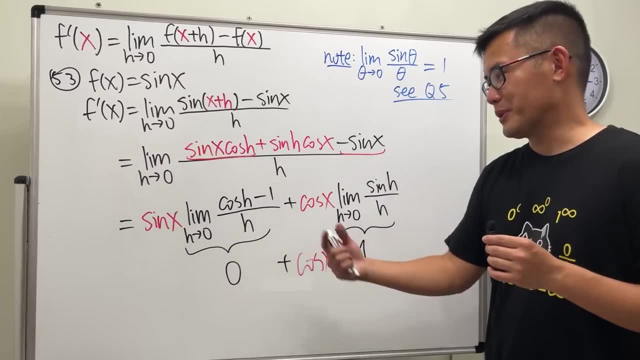 and bottom by conjugate and use this to help you out. You can try it, But I will tell you the answer right here. You get 0.. Or you can use the graph. Just use the graph. Use the calculator, Plug in. 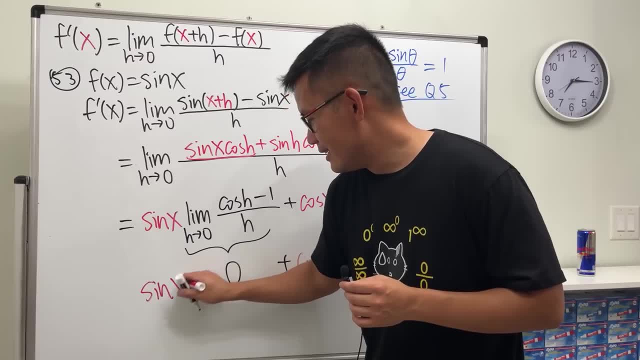 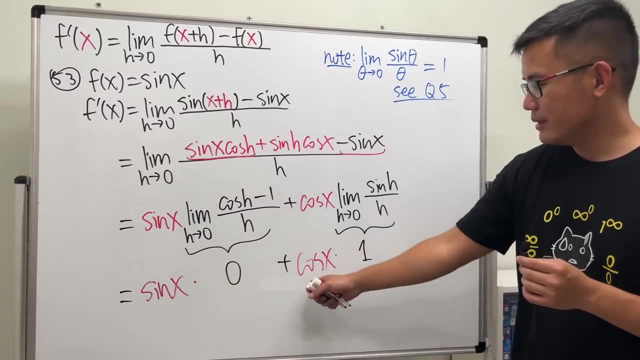 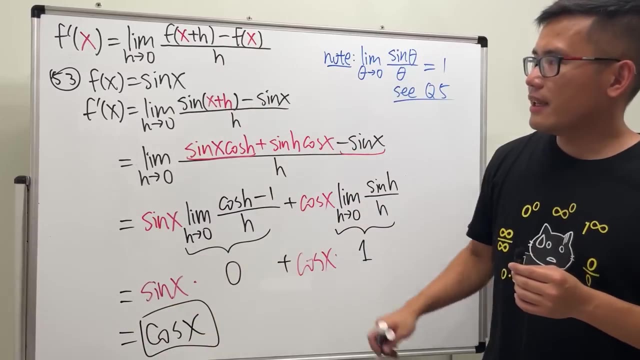 the numbers. That's not a discussion For here, But like that's equal to 0.. So only we get what 0 cosine x? Hey, the answer is just nicely equal to cosine x, Sine and cosine. 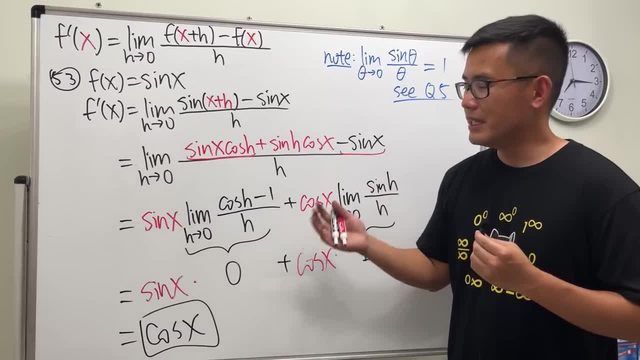 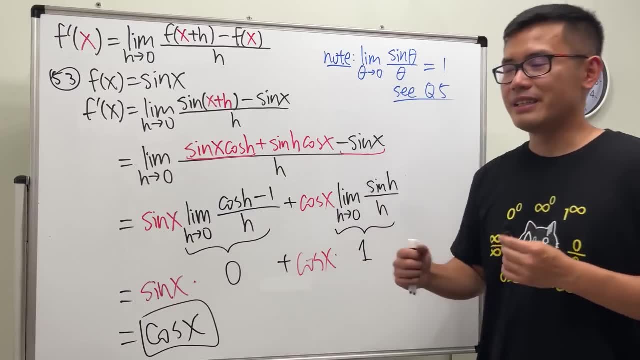 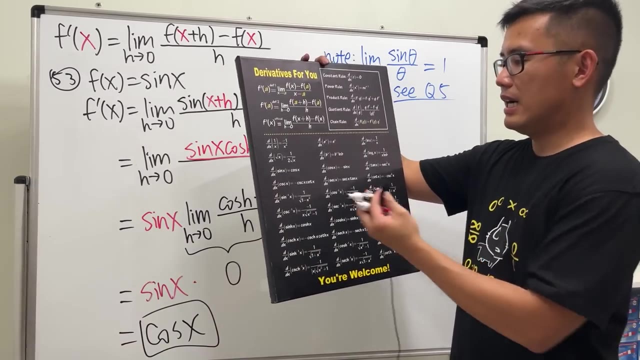 Yeah, They're always together In precalc, trig and also calculus, of course. Yeah, They don't run away from each other. Yeah, And let me just make sure that it is right. Aha, Derivative of sine x is equal to cosine x. 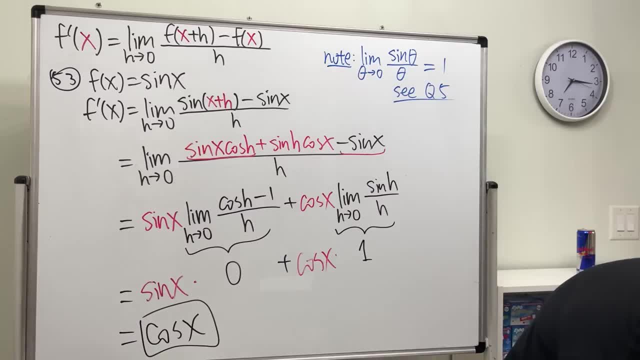 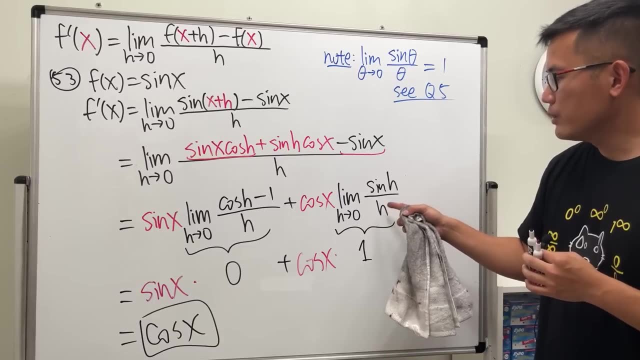 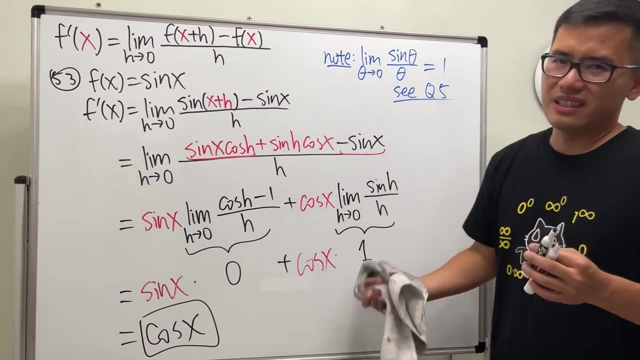 Told you Okay. Anyway, I want you guys to pay attention to that. Hey, we run into this limit right here when we are trying to get the derivative of sine x. This is going to show up later on Like an hour. 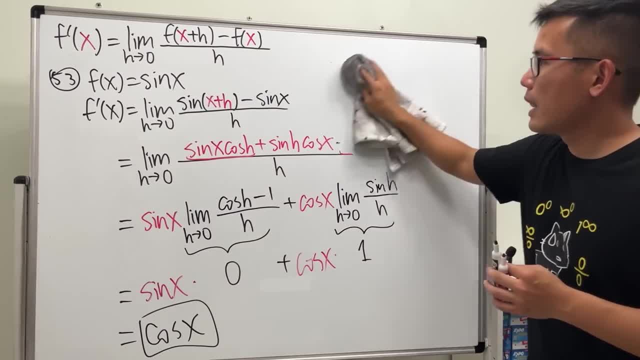 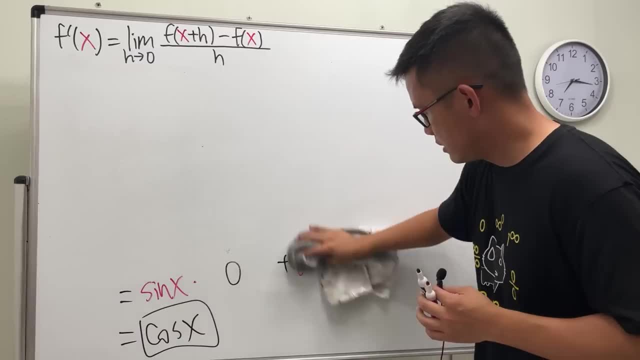 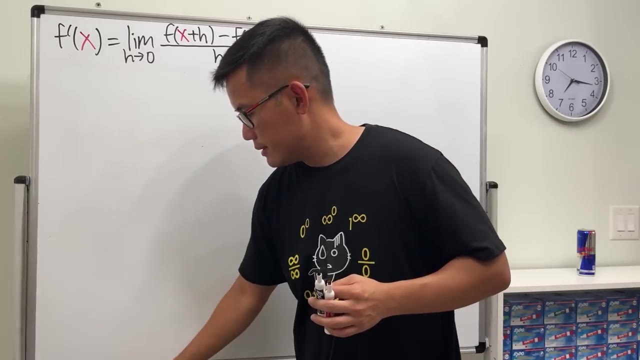 or two, I don't know. By the way, I'm going to take a look at 54.. All right, So now let's take a look at 54.. Here we have the- Sorry, We are still doing the definition of. 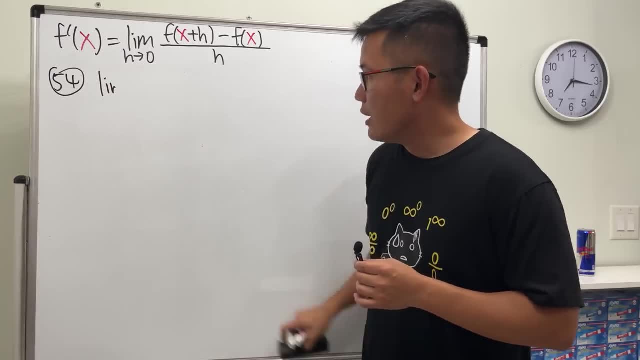 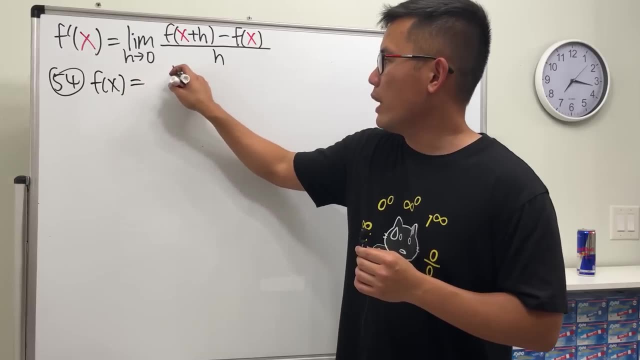 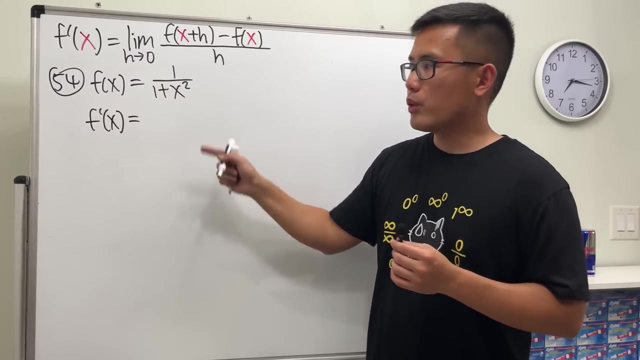 derivative, Number 54, we have the derivative of sine x, We have the function f of x. This is 1 over 1 plus x squared, and then we want f prime of x. Can we use the power rule right here and say the answer is: 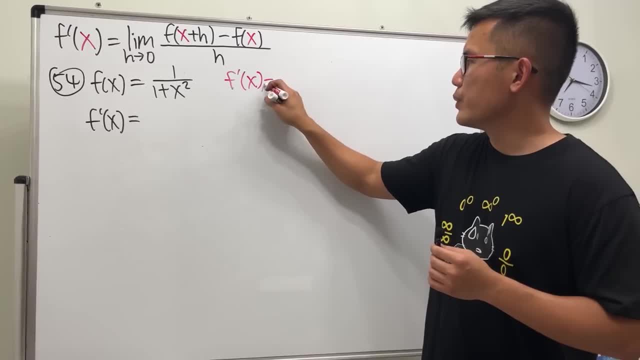 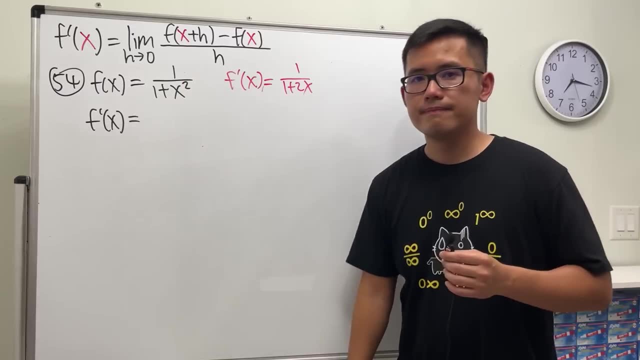 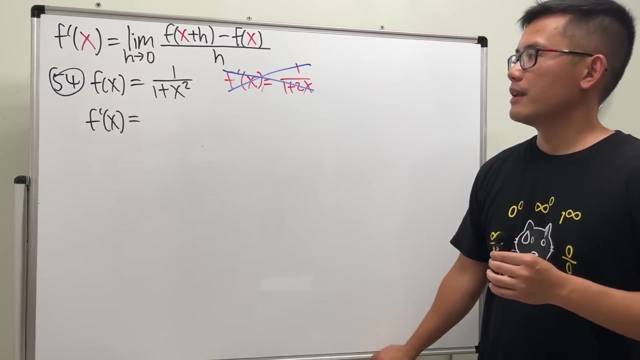 f prime of x equals to the power rule, and then we get 1 over 1 plus 2x. Can we Putting the 2 to the front minus 1?? No, Right, No, I will show you we can actually. 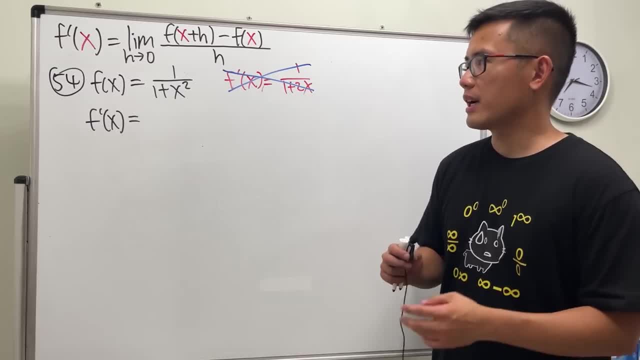 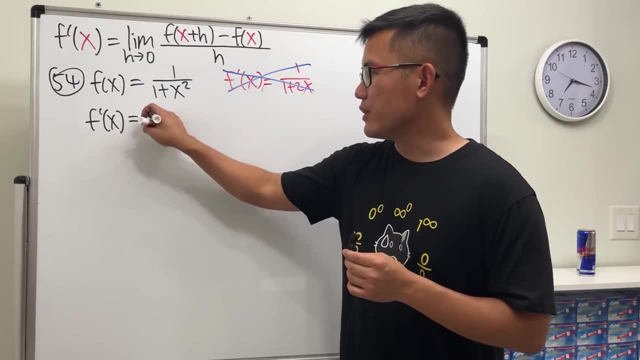 use the power rule along with something called the chain rule, and then we can actually still formulate the easy way, aka the so-called easy way to do this kind of question. But let's do the definition of derivative first. The limit is h approaching 0,. 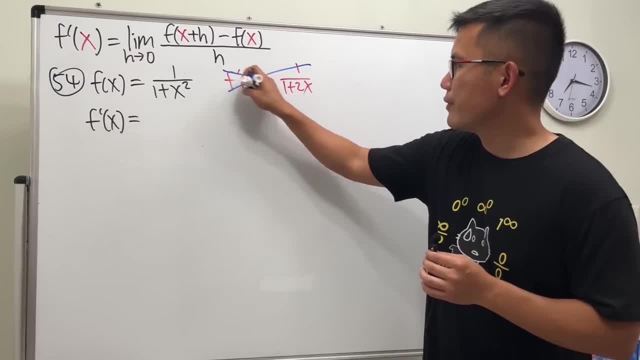 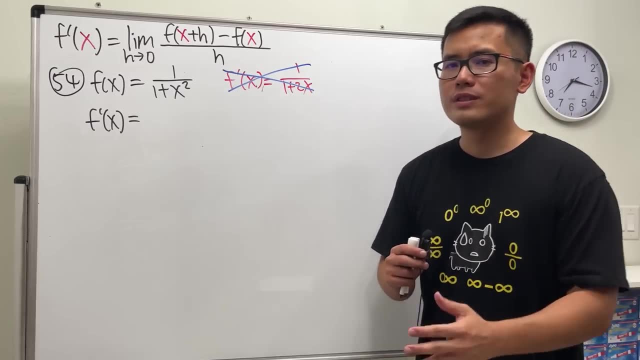 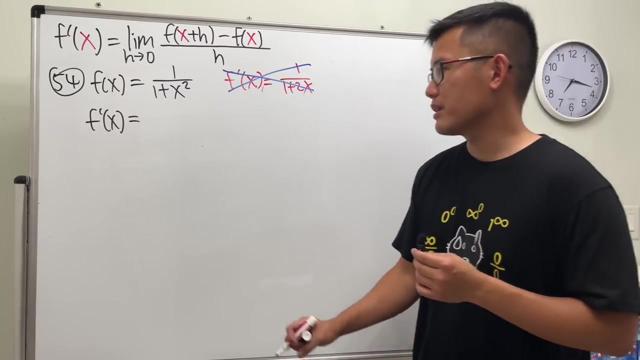 no, right? no, i will show you we can actually use the power rule along with something called the chain rule, and then we can actually still formulate the easy way, the, aka the so-called easy way to do this kind of question. but let's do the definition of the remedy first. the limit as h approaching 0. 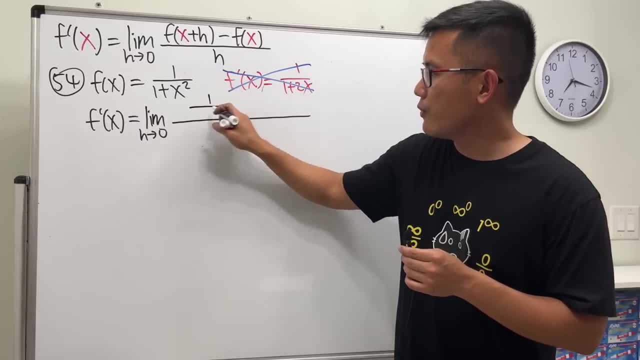 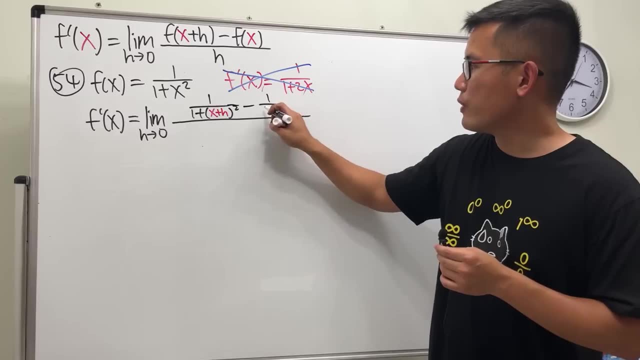 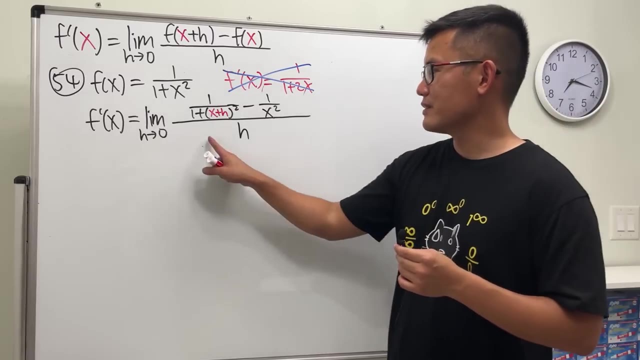 f of x plus h. so we put that here: 1 over 1, plus parentheses, x plus h, and then we square that and then minus 1 over x, squared and over h. wow, it's a complex fraction with a lot of things. anyway, multiply the top and bottom by this and that so 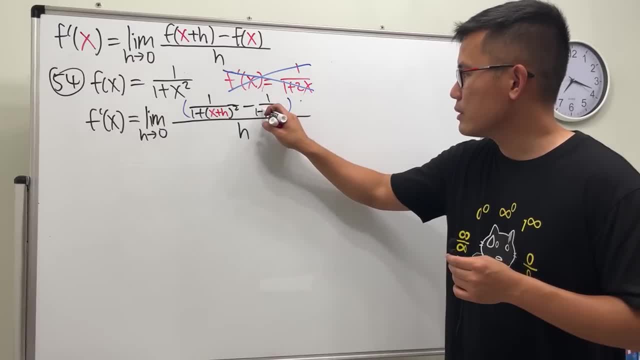 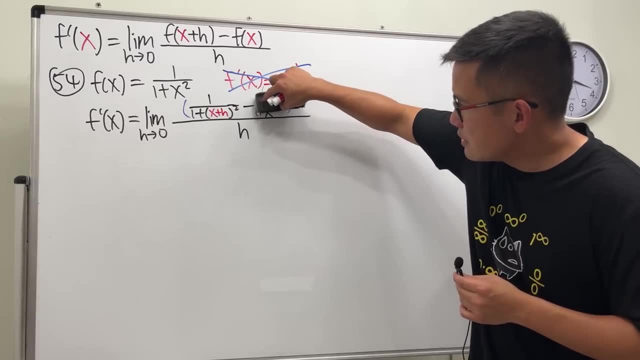 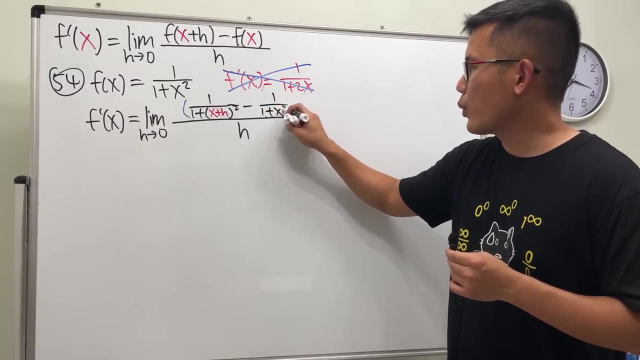 oh sorry, it's not just x squared, it's 1 plus x squared. wow crazy. uh, hope you guys can see this. okay, let me just fix this a little bit. one over one plus x squared ready. multiply the top and bottom by this, which is 1 plus x squared. 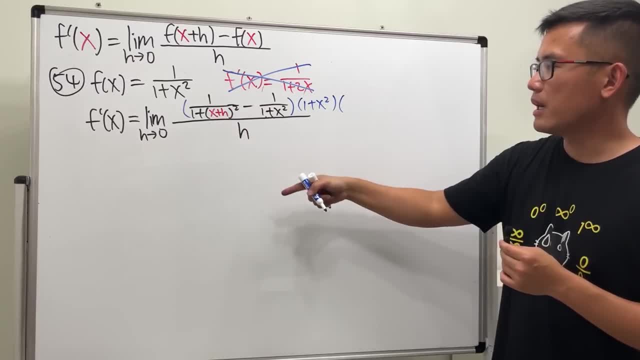 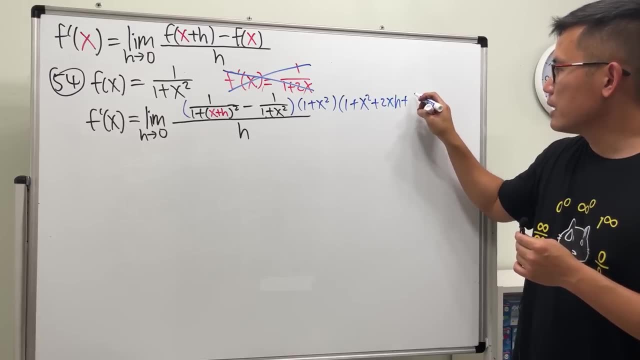 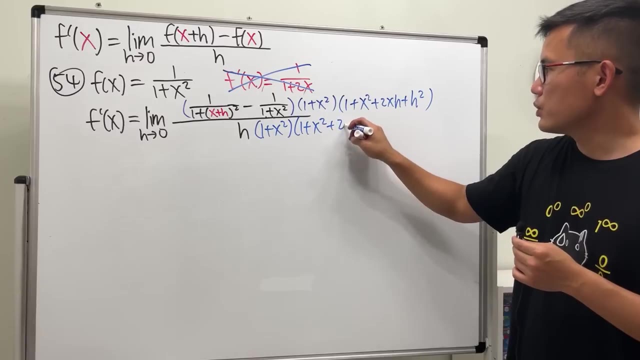 also that, and perhaps i'll just multiply this out right here at the same time. so we have 1 plus open, that we get x squared plus 2x h plus h squared, and then, of course, let's also put that down on the bottom here: 1 plus x squared plus 2x h plus h squared. 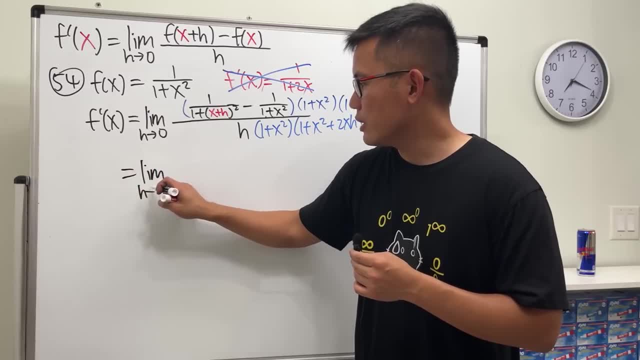 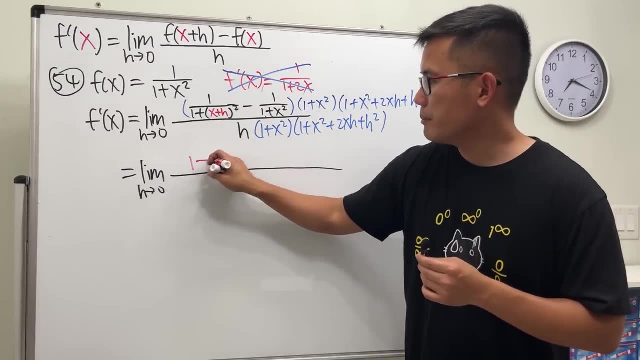 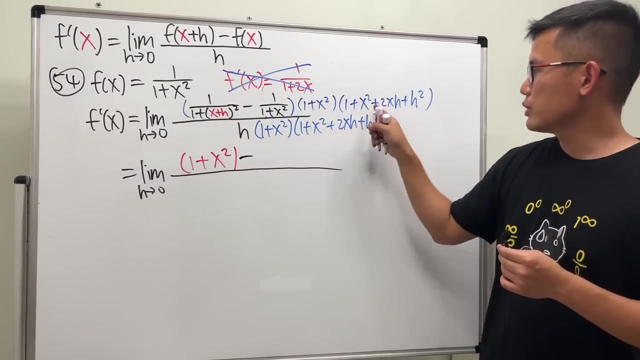 all right. so here we will have the limit as h approaching zero. take this times that this and that cancel. so we have the first part, 1 plus x squared and then minus. this times that this and that cancel. so we just have this. so i'm just going to keep it. 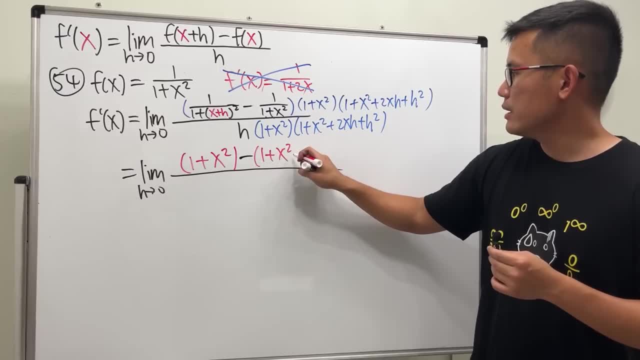 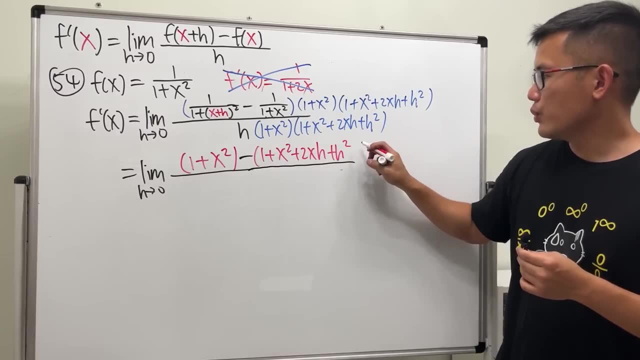 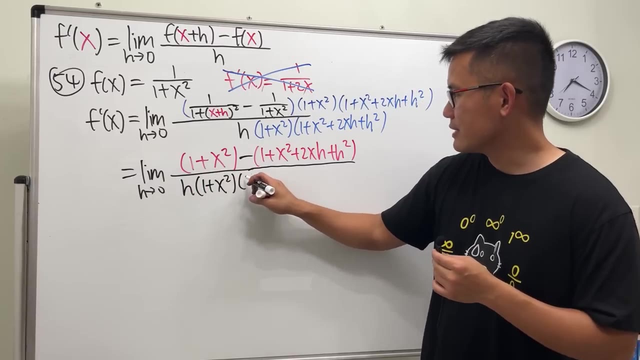 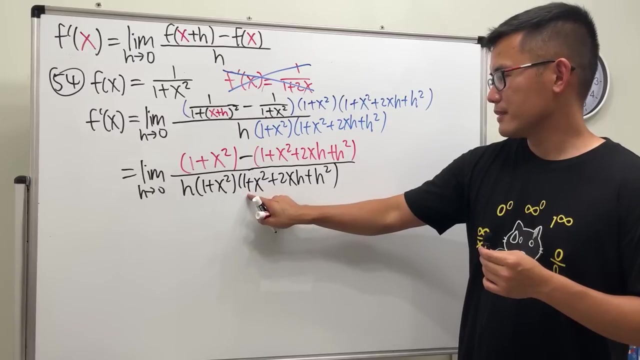 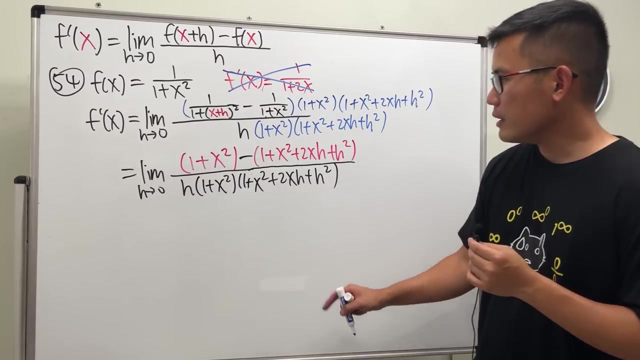 in the parentheses, we get 1 plus x squared, plus 2x h plus h squared. all right, cool. and then the bottom maintain it: h times 1 plus x squared. times 1 plus x squared, plus 2x h plus h squared. wow, i wish i could just copy and paste. maybe it's easier that way. huh, anyway, so we're just going to. 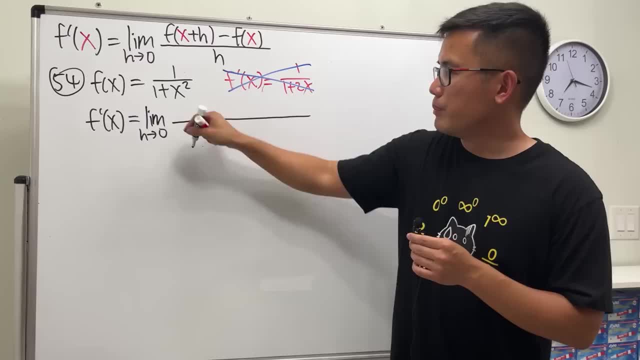 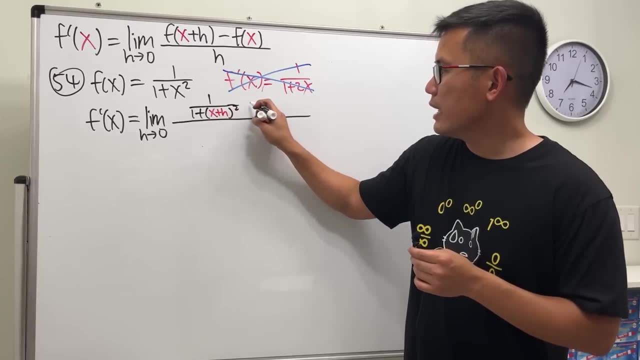 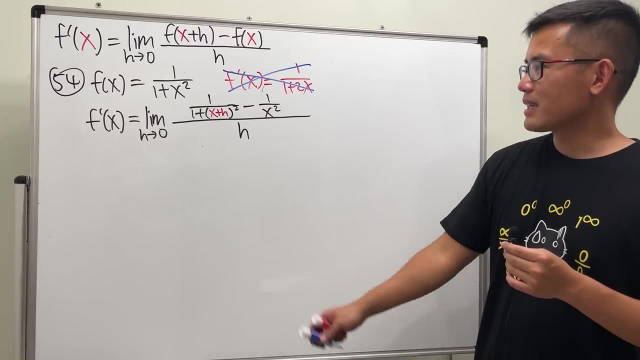 f of x plus h. so we put that here: 1 over 1 plus parentheses, x plus h, and then we square that and then minus 1 over x squared, and then over h. Wow, It's a complex fraction with a lot of things. 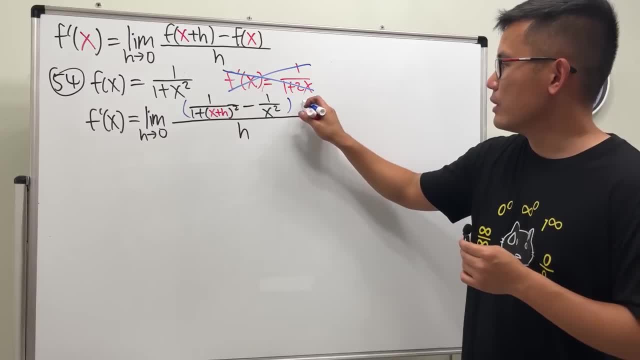 Anyway, multiply the top and bottom by this and that, so, oh sorry, it's not just x squared, it's 1 plus x squared. Wow Crazy. I hope you guys can see this. Okay, let me just fix this a little bit. 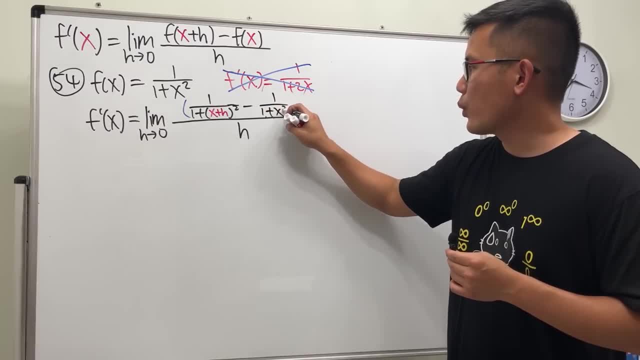 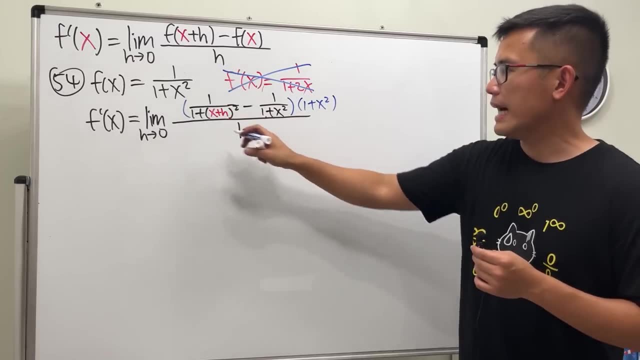 1 over 1 plus x squared Ready. Multiply the top and bottom by this, which is 1 plus x, squared also that, and perhaps I'll just multiply this out right here at the same time. so we have 1 plus open that. 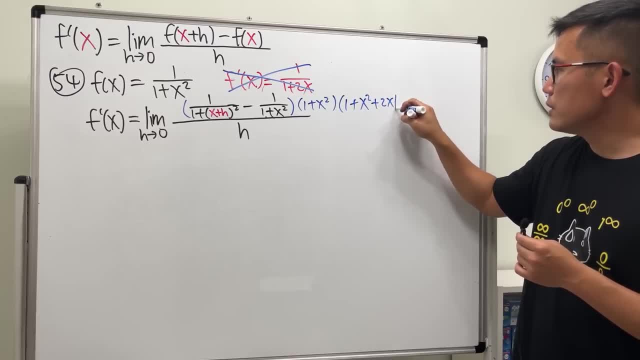 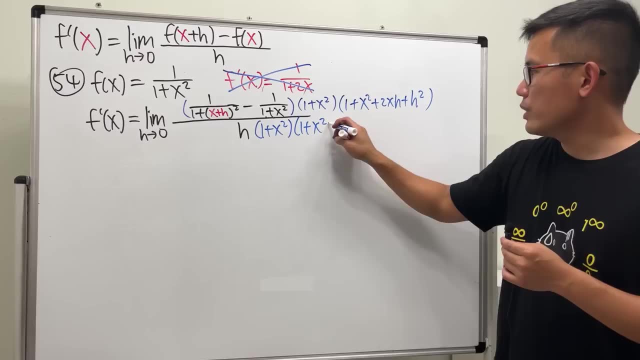 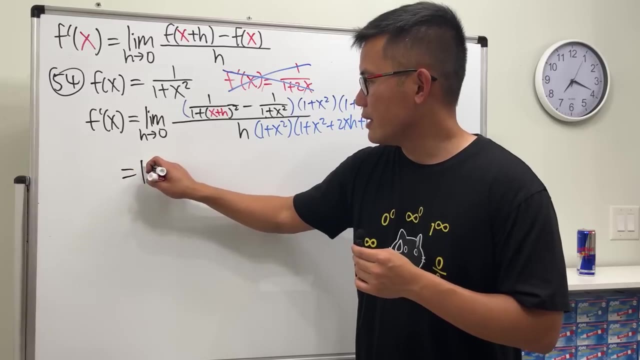 we get x squared plus 2xh plus h squared, And then, of course, let's also put that down on the bottom here: 1 plus x squared plus 2xh plus h squared, Alright, so here we will have the. 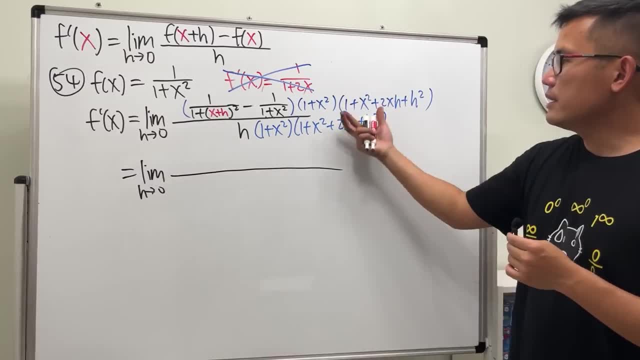 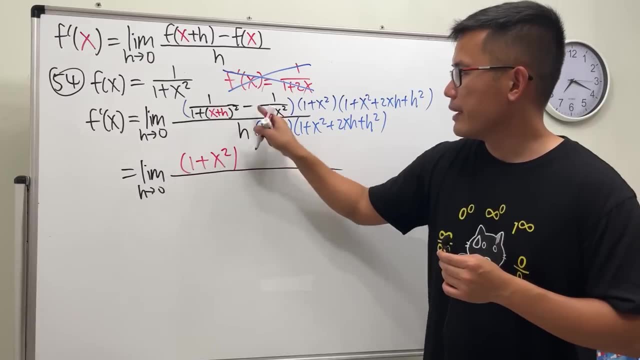 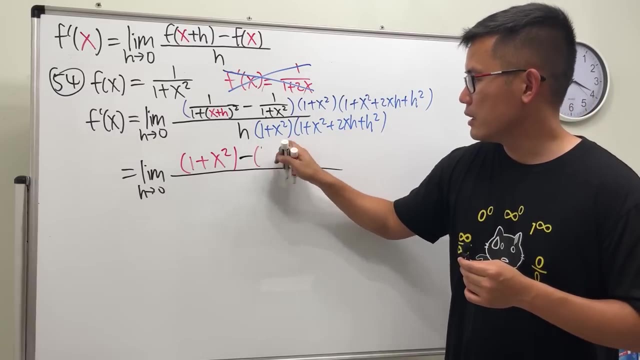 limit as h approaching 0.. Take this times that This and that cancel, so we have the first part, 1 plus x squared And then minus This times that This and that cancel, so we just have this. So I'm just going to keep it in the parentheses. 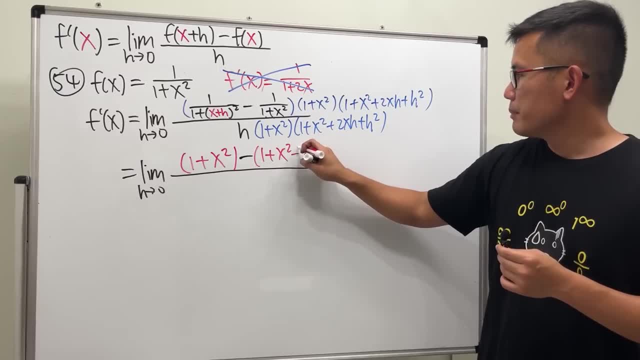 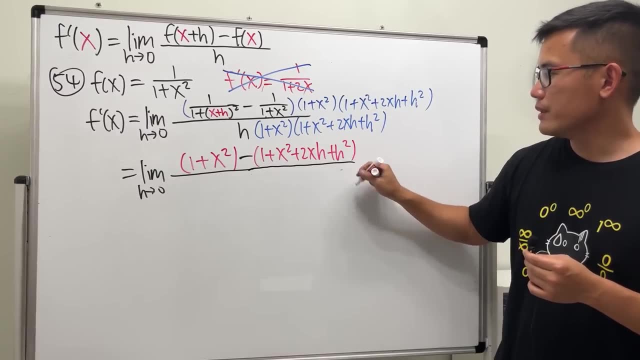 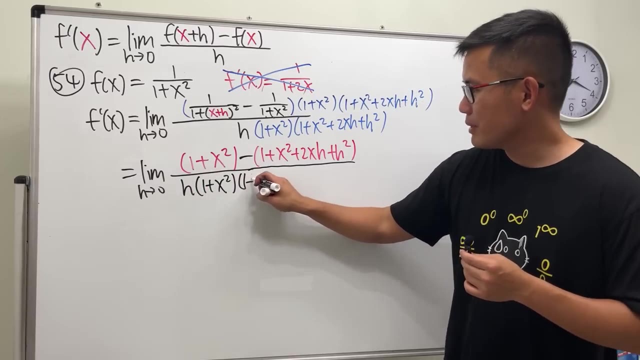 We get 1 plus x squared, plus 2xh plus h squared. Alright, Cool. And then the bottom maintain it: h times 1 plus x squared times 1 plus x squared, plus 2xh plus h squared- Wow. 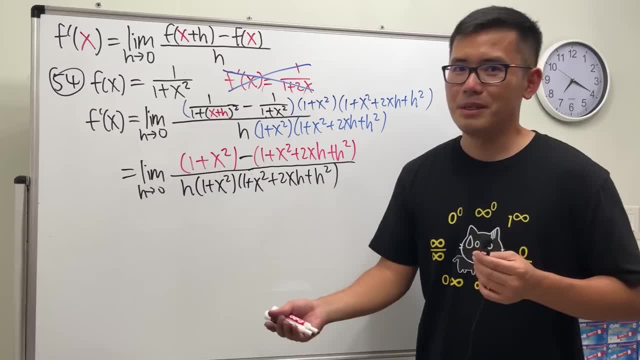 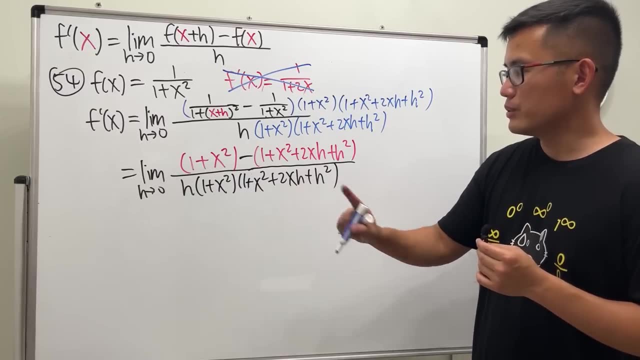 I wish I could just copy and paste. Maybe it's easier that way, huh, Anyway. so we're just going to see what we can do. Check this out: 1 minus 1.. This and that. cancel yeah, 1 minus 1, because you have to. 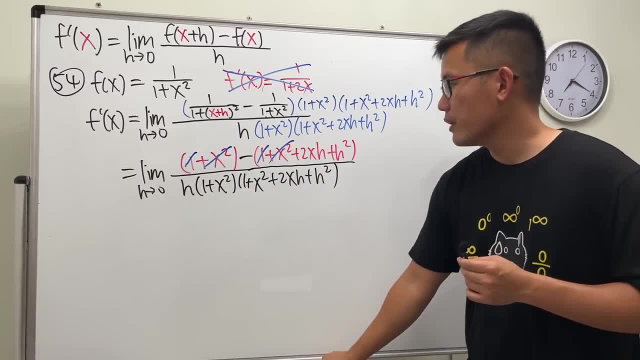 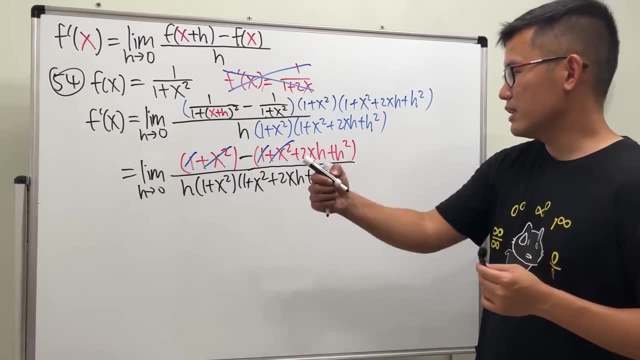 distribute the 1. And x squared, x squared, cancel. So you see that we just have this and that left And they both have h. We can factor that out And it has a negative in the front. Let's keep the negative in the front as well. 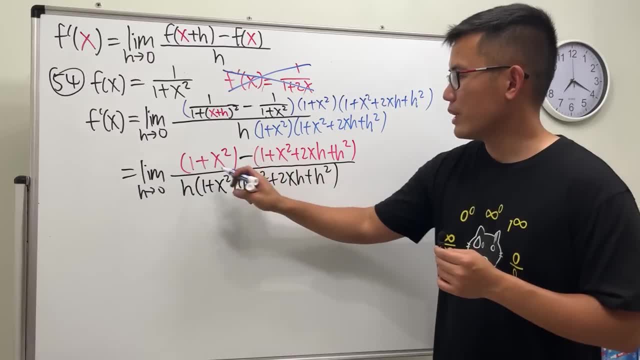 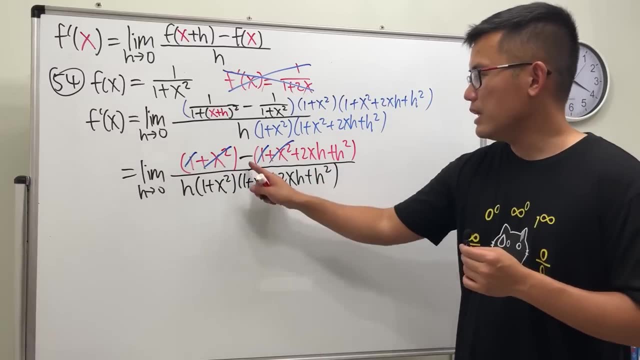 see what we can do: check this out, 1 minus 1, this and that and cancel. yeah, 1 minus 1, because you have to distribute the 1 and then x squared, x squared, cancel. so you see that we just have this and that left and they both have h. we can factor that out and it has a negative in the front. let's 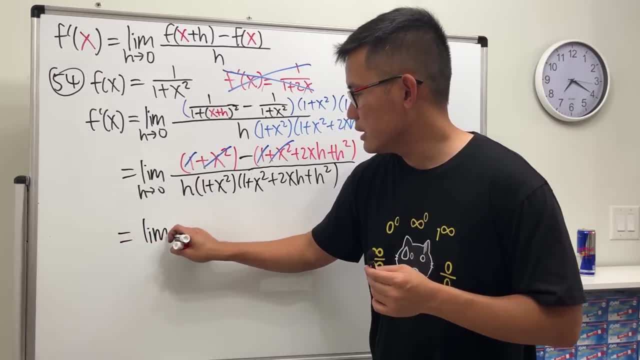 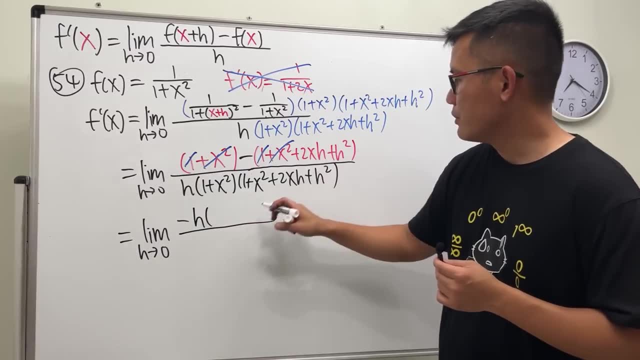 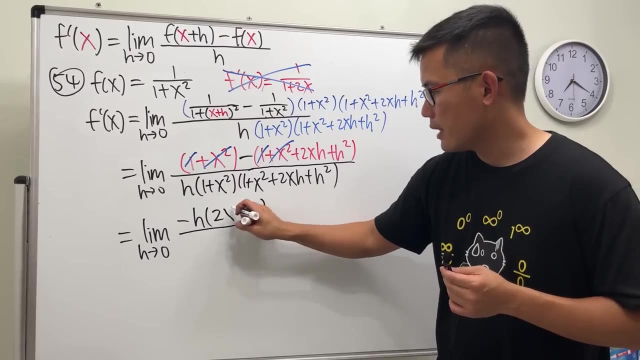 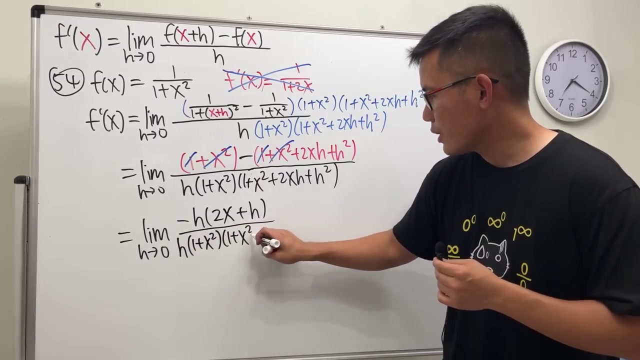 keep the negative in the front as well. so we have the limit as h approaching zero, negative h on outside, and then we have 2x plus another h, like, so, like, so, all right, and then all that stuff: h times 1 plus x squared times 1 plus x squared. 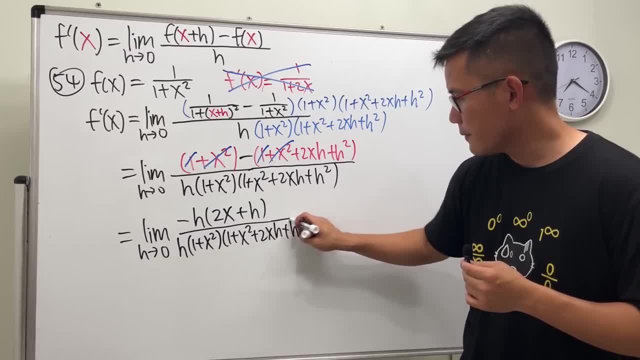 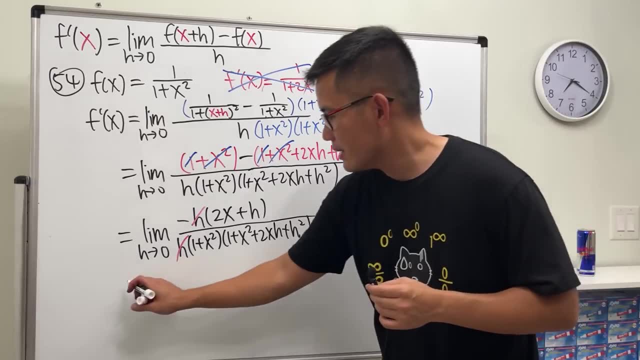 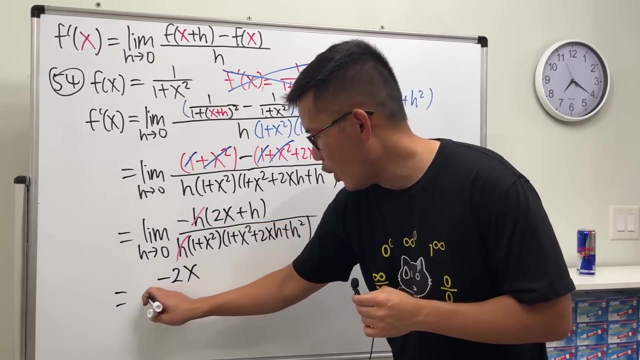 plus 2xh plus h squared. yay, okay, let's do this in our head: puts 0 into h. right, puts 0 into h, so we have negative 2x on the top over. here we have what: 1 plus x squared. 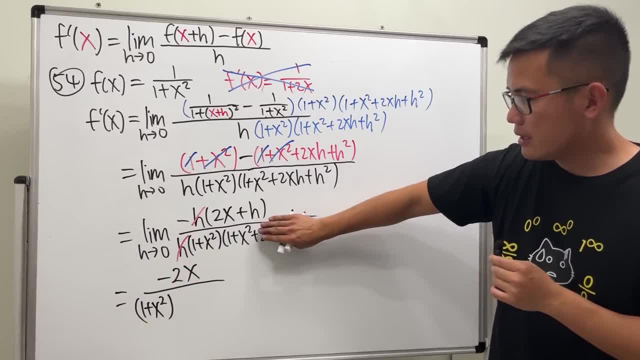 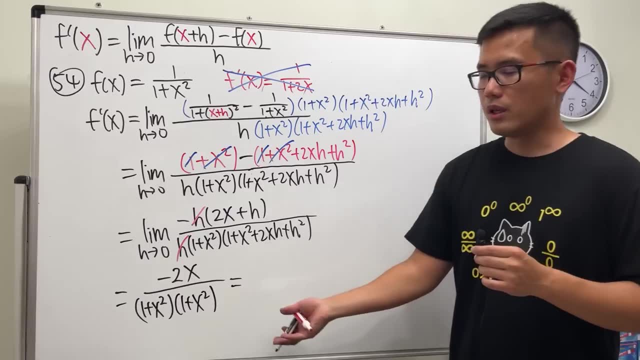 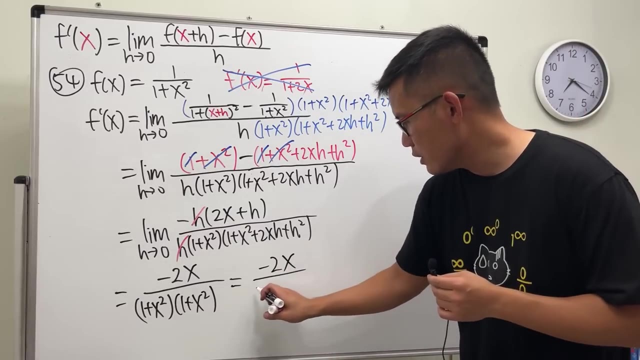 all right, and then put 0 into h, so this and that cancel. we have 1 plus x squared. whoa, look at that. it's a pretty clean result. this and that are the same, though, so we can just put it as power 2, right, so negative 2x over 1 plus x squared, and then 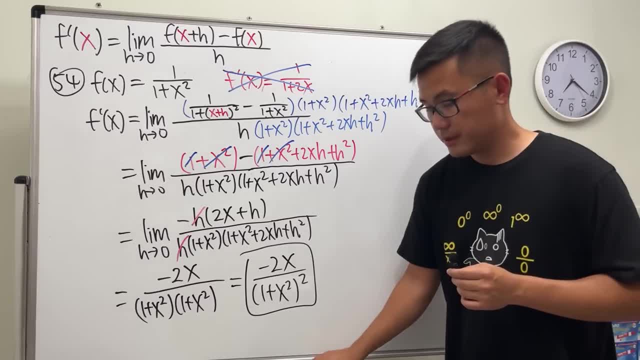 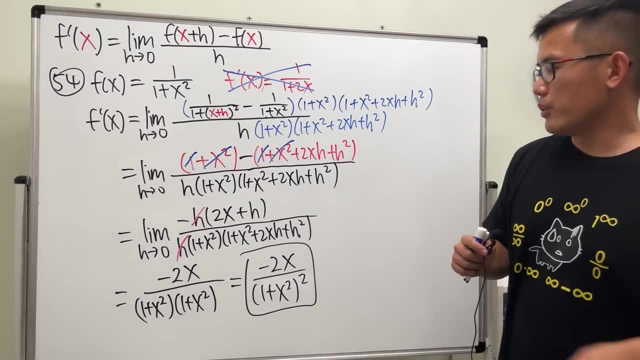 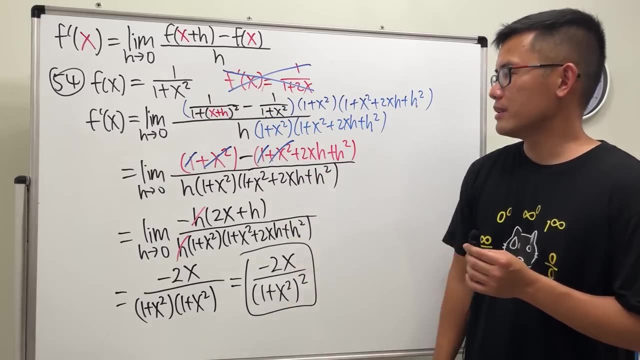 we are done, cool. okay now, as promised earlier, I told you guys we can use the power rule and you see this is totally wrong. but how can we really avoid doing the definition of derivative? check this out- it's all about rewriting- and then also pay attention to. 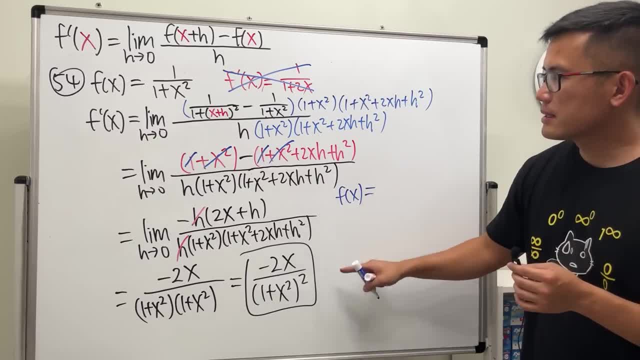 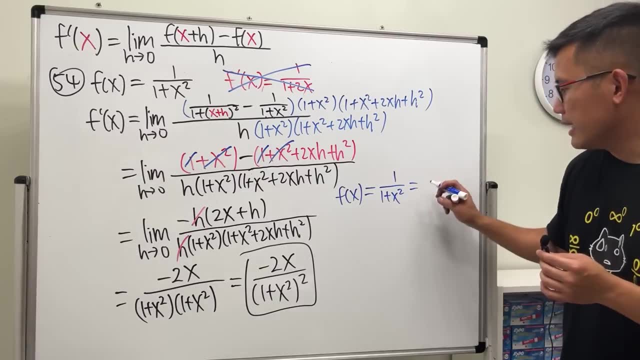 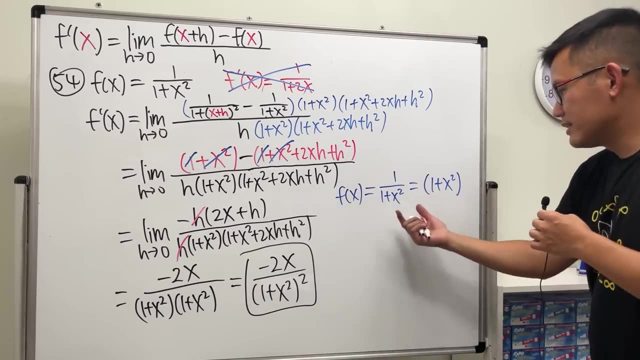 the so-called chain rule f of x is that 1 over 1 plus x squared, and then we have 1 plus x squared. let's first purposely rewrite this as parentheses, with 1 plus x squared inside, but then, because we bring up, we brought this up right, so it will be the. 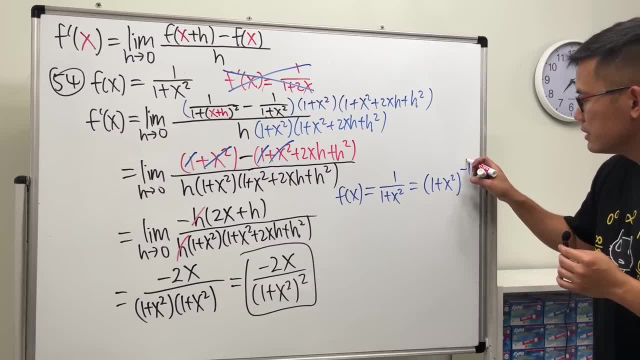 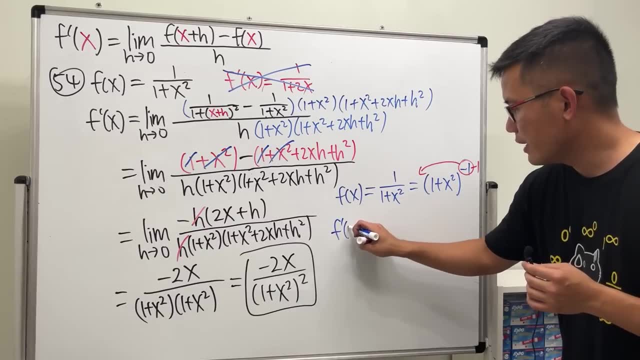 negative 1 power, and the reason now we want to do this is now we can use the power rule. bring the power to the front and then minus 1, what do we get? f, prime of x, we have the negative right here, and then the base. 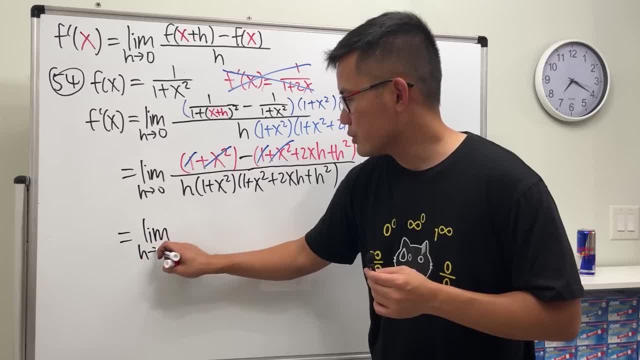 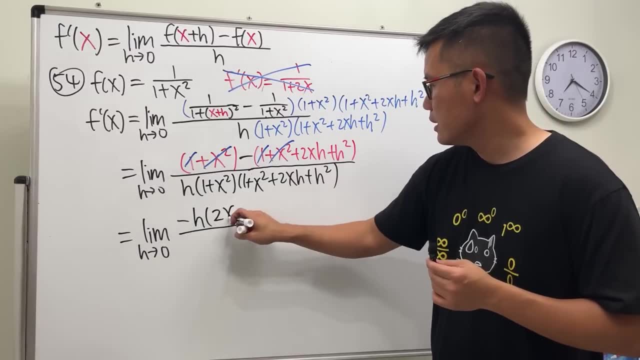 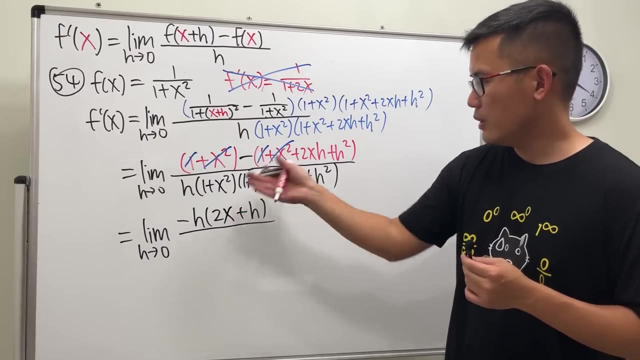 So we have the limit as h approaching 0.. Negative h on the outside, And then we have 2x plus another h, like so, Alright, And then all that stuff, h times 1 plus x squared times 1 plus x squared plus. 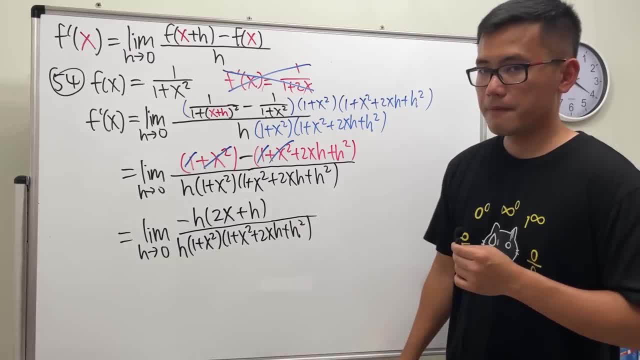 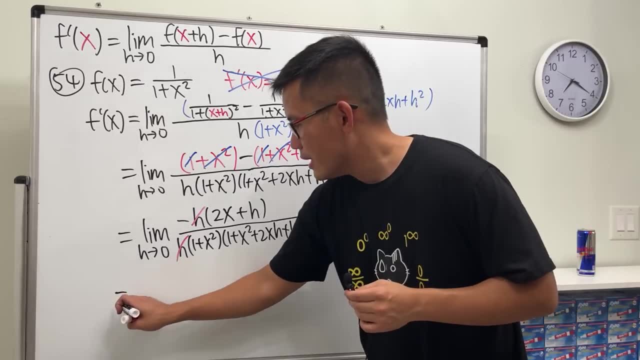 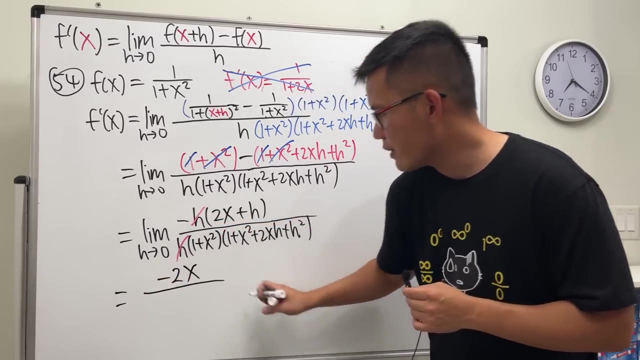 2xh plus h squared. Yay, Okay, Let's do this in our head: Put 0 into h. Alright, Put 0 into h, So we have negative 2x on the top Over Here we have what. 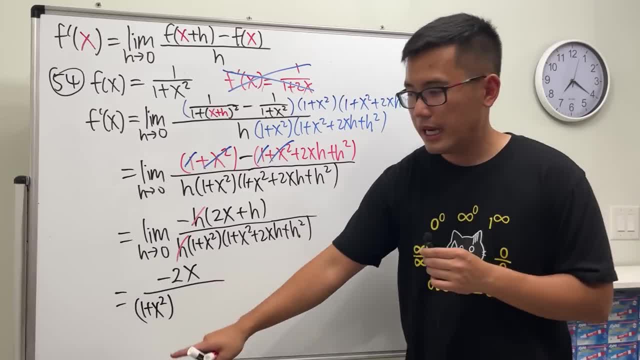 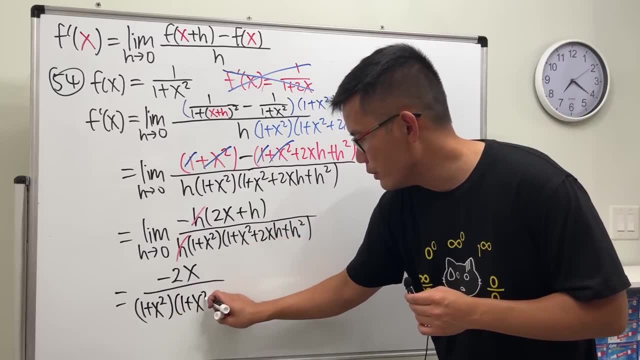 1 plus x squared- Alright, And then put 0 into h, So this and that cancel. We have 1 plus x squared. Wow, Look at that. It's a pretty clean result. This and that are the same, though, So we can just. 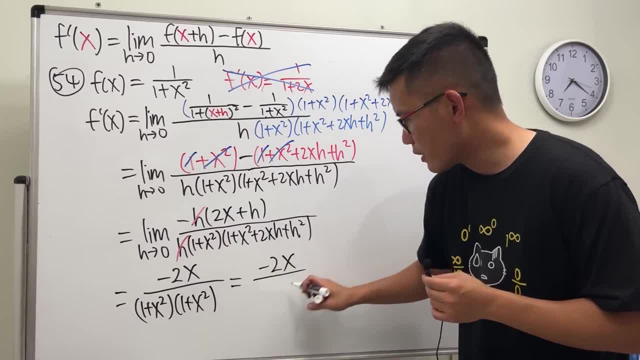 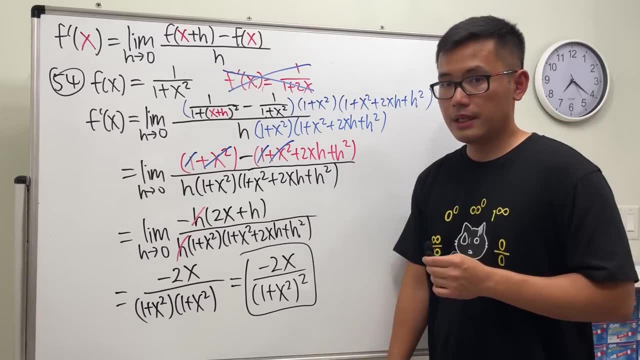 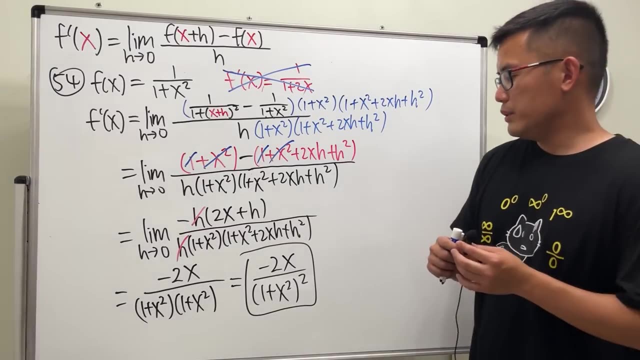 put it as power 2, right, So negative 2x over 1 plus x, squared and then squared, And then we are done. Cool, Okay. Now, as promised earlier, I told you guys we can use the power rule, And you see. 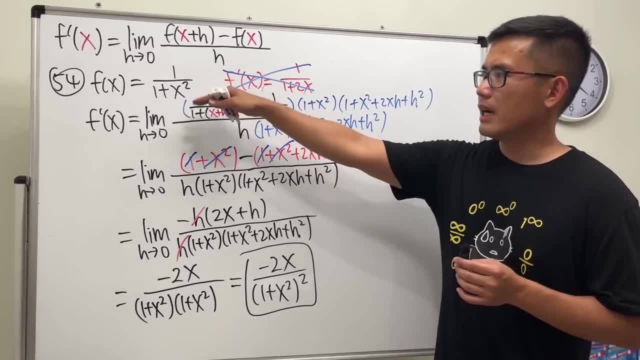 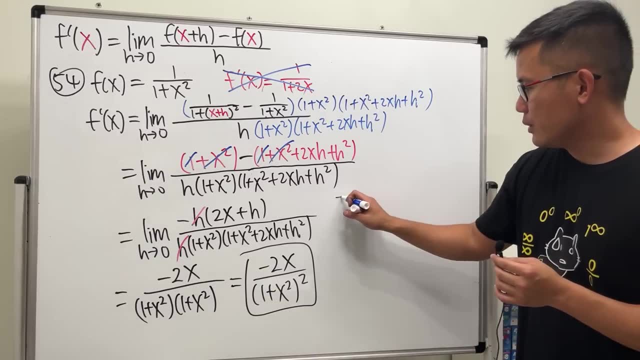 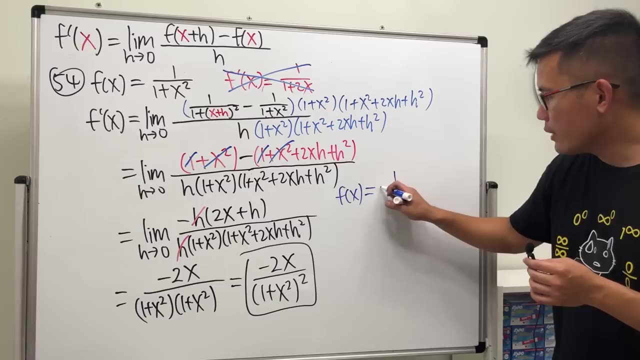 this is totally wrong. But how can we really avoid doing the definition of derivative? Check this out- It's all about rewriting- and then also pay attention to the so-called chain rule f of x. is that 1 over 1 plus x squared? 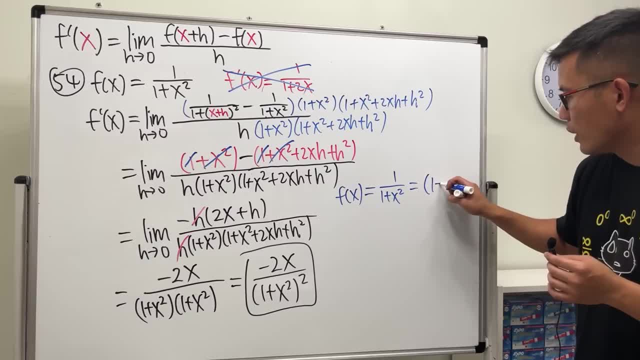 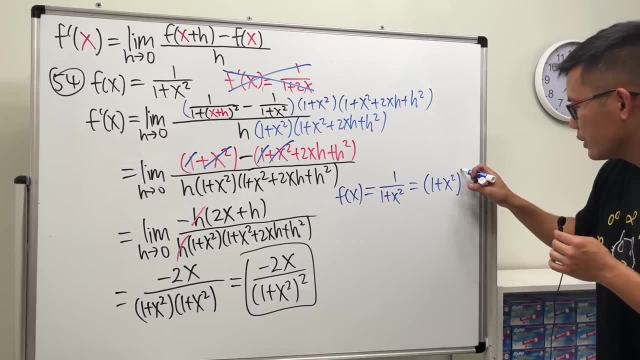 Let's first purposely rewrite this as parentheses, with 1 plus x squared inside, But then, because we bring up, we brought this up right, So it will be the negative 1 power. And the reason now we want to do this is now we can use the power rule. 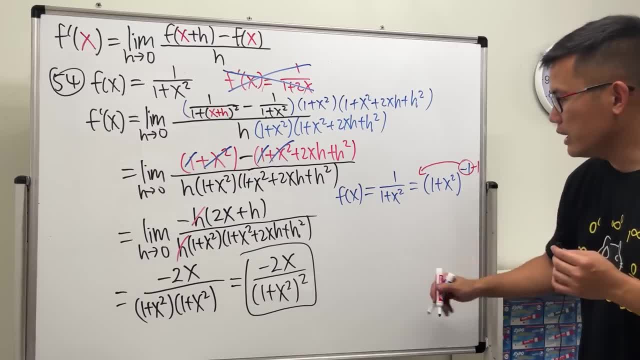 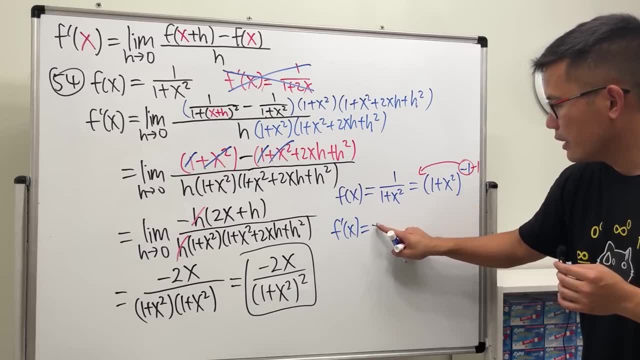 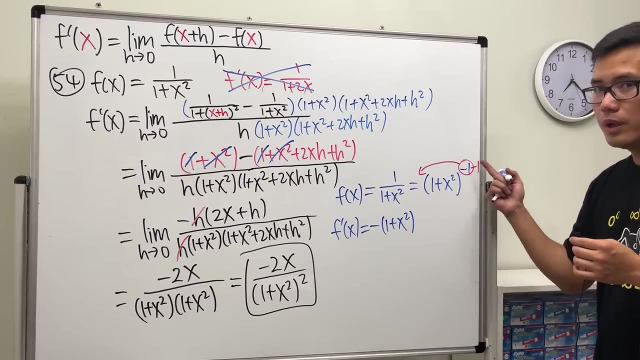 Bring the power to the front and then minus 1.. What do we get? f prime of x. We have the negative right here And then the base. you keep it, which is 1 plus x squared, and the negative, 1 minus 1. 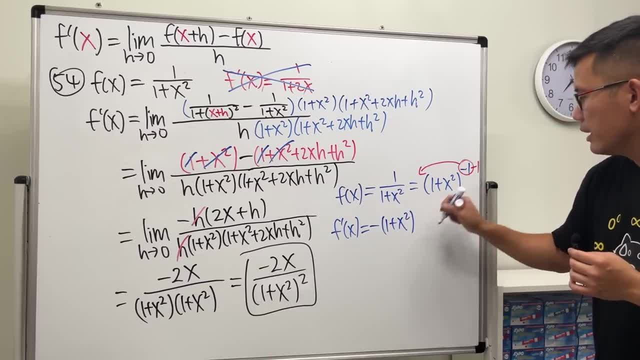 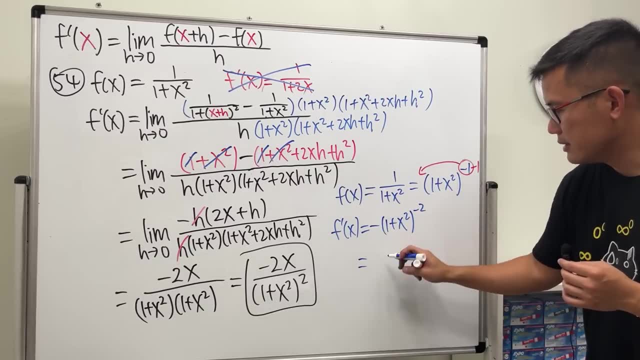 you keep it, which is 1 plus x squared, and then 1 minus. well, negative 1 minus 1 is negative 2, okay, wow, look, I can bring this down to the bottom and this is negative 1. 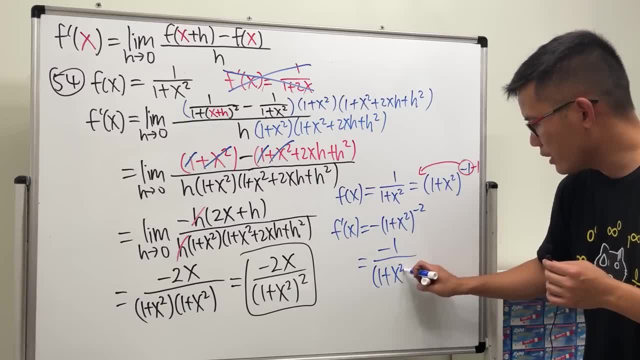 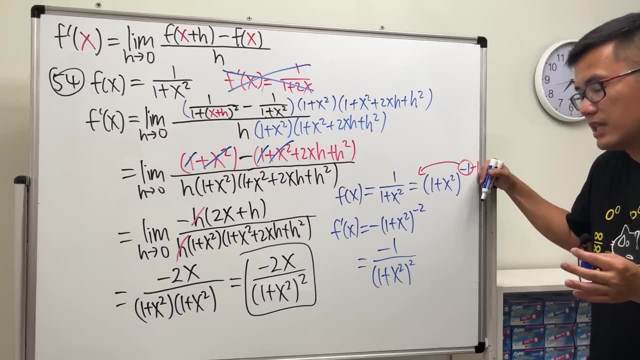 over. this is 1 plus x, squared and then squared. wait, I thought we can use, I thought we could use the power rule, but I can't, I can't, I can't. I get negative 1 on the top right here. earlier we have negative 2x. what's the deal? 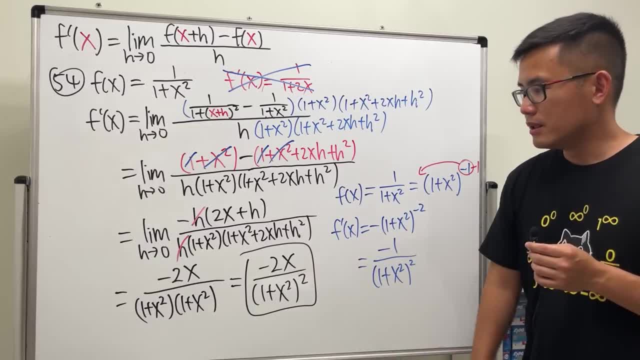 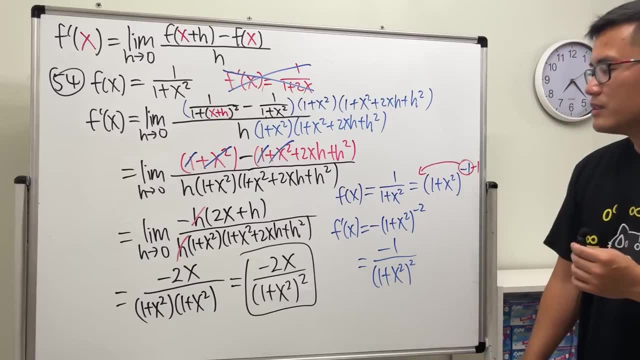 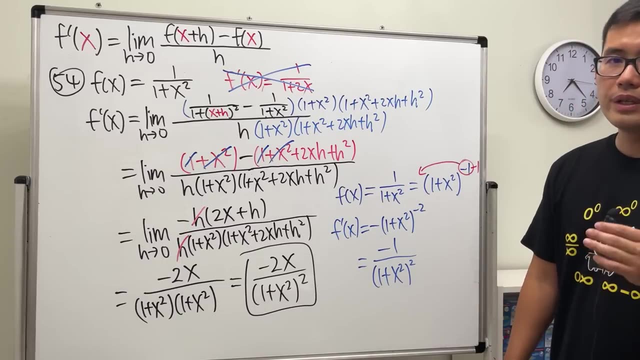 is that wrong? that's wrong. it must be wrong. the easy way is always right. no definition is much better. stall it. so here's the deal. how can we come up with the 2x? well, we're in calculus, so we have to think derivative. here's the deal. when we put the 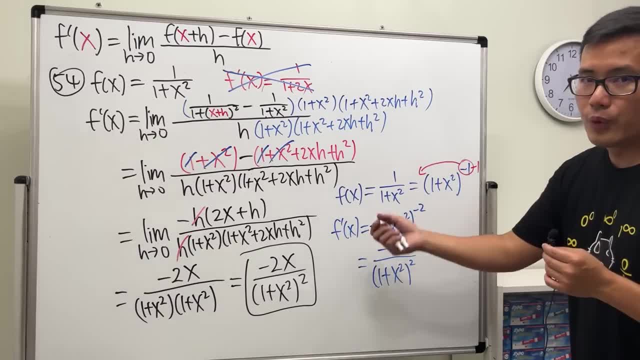 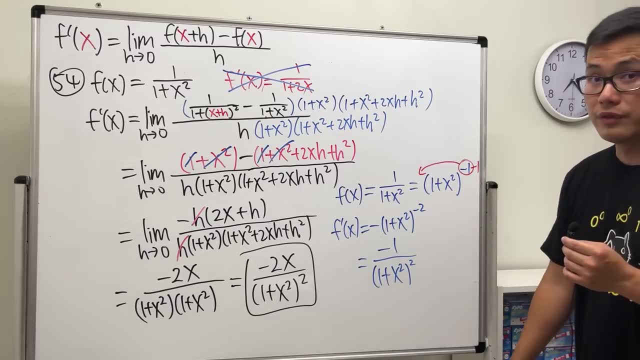 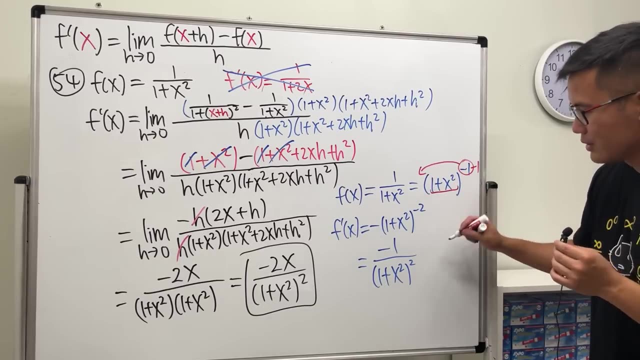 the negative 1 to the front and then minus 1. we just do the power on the outside and the idea is you also have to look at inside to see what the function is and multiply the derivative of that. so you see the derivative of this. the derivative of 1 is 0, but the derivative of x squared is 2x. 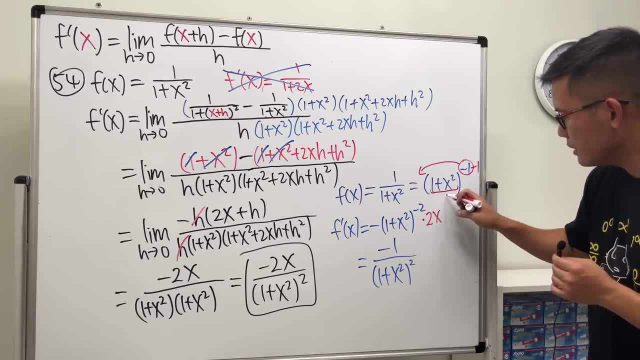 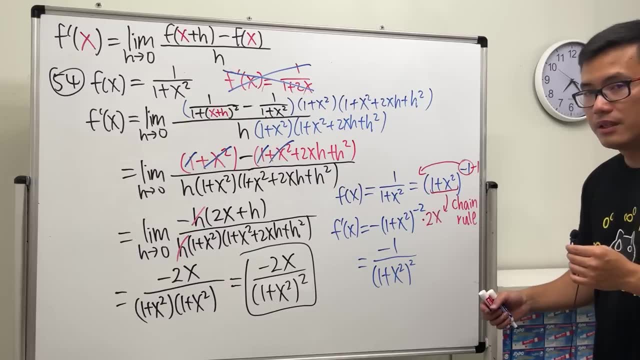 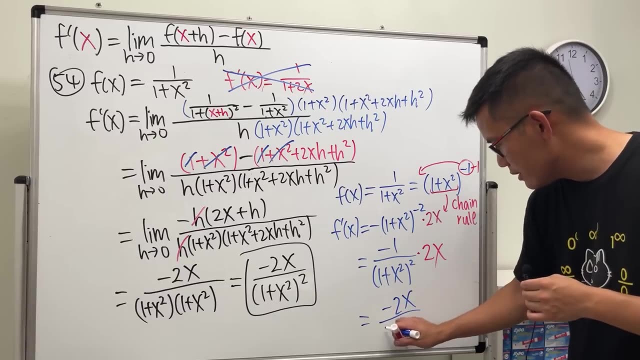 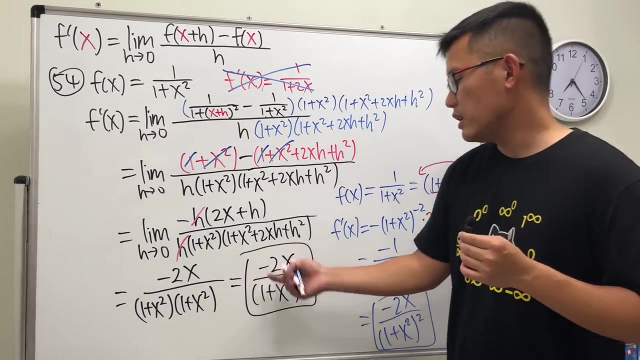 so we have to multiply this by 2x. so this is the so-called chain rule part which is needed. so you see, if we multiply by 2x altogether we have the answer that we have earlier. so hopefully you guys can see why we need the definition of derivative. it tells you: 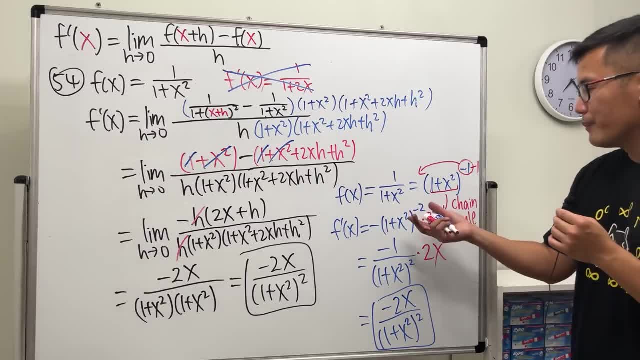 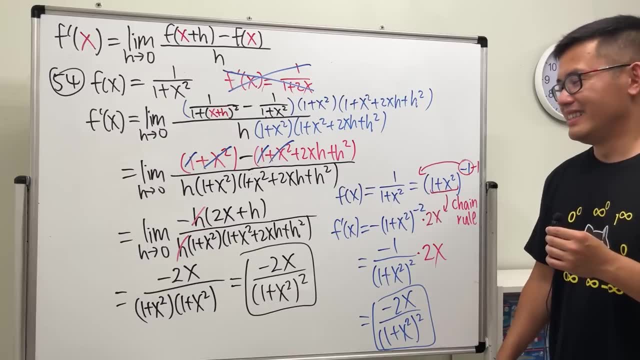 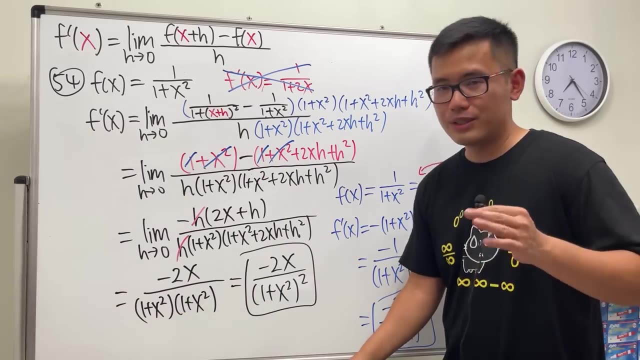 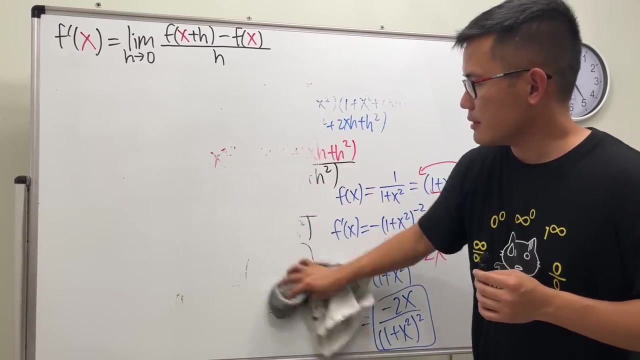 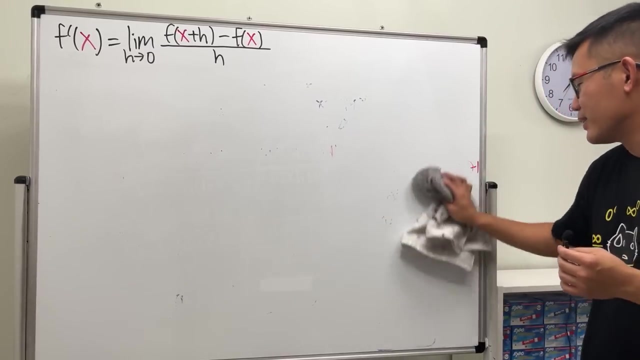 what has to be right. if you want to use the shortcut well earlier without seeing that, then we'll miss the 2x right. so that's the reason for the definition of derivative. and then that's do it again for number 55.. and maybe you guys can count how many times have i said, have i said: here's the deal, i, i don't. 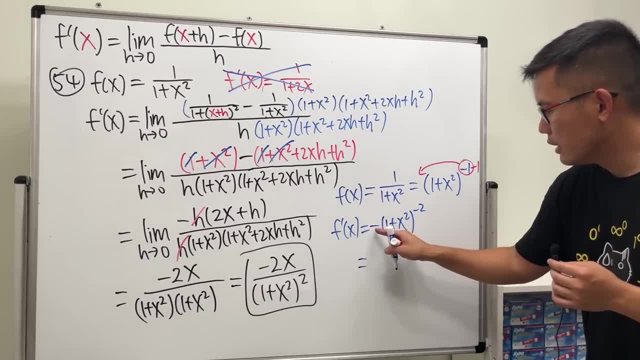 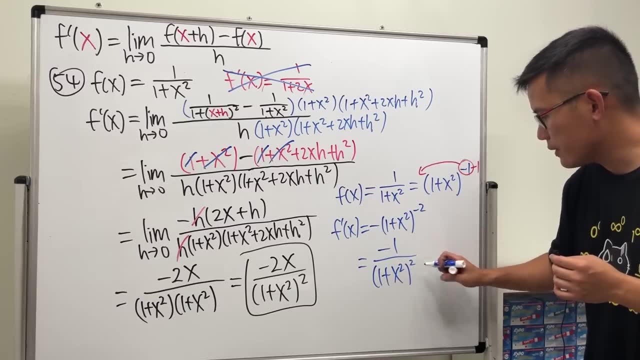 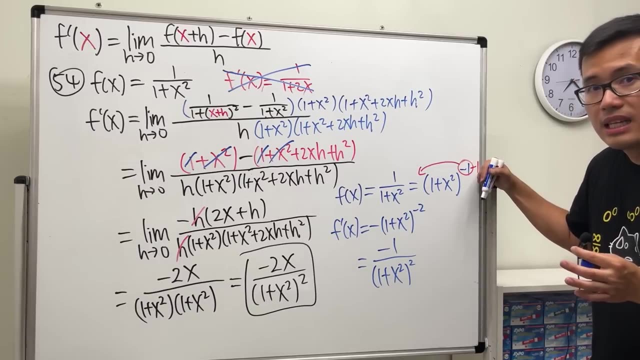 is negative 2.. Okay, Wow, Look, I can bring this down to the bottom. and this is negative 1 over. This is 1 plus x, squared and then squared. Wait, I thought we can use, I thought we could use the power rule. 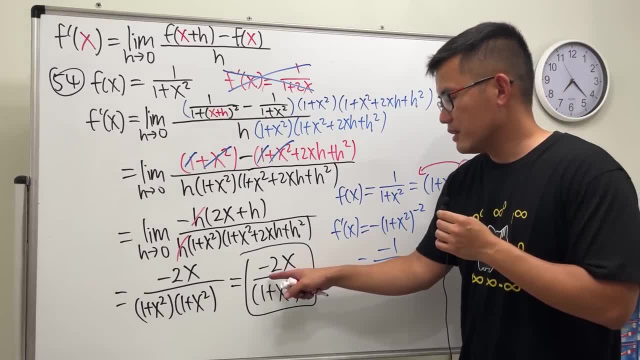 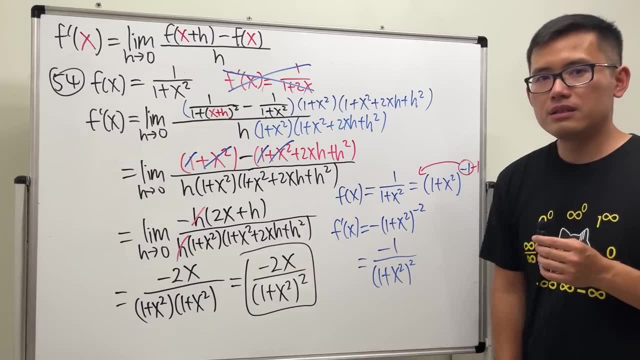 But I get negative 1 on the top right here. Earlier we have negative 2x. What's the deal? Is that wrong? That's wrong. huh, It must be wrong. The easy way is always right, huh, No. 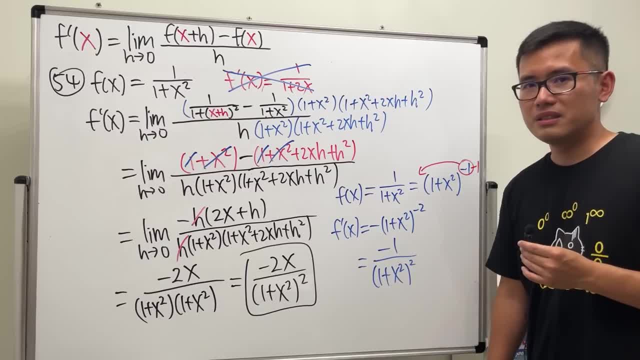 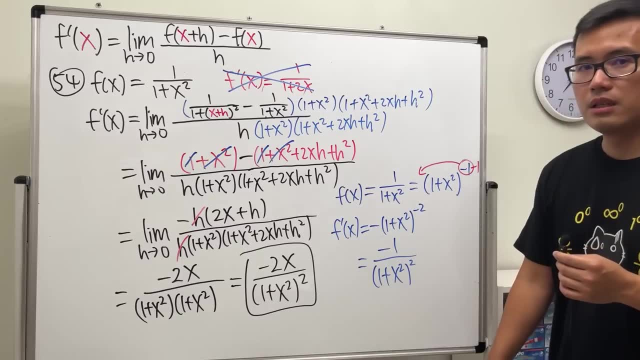 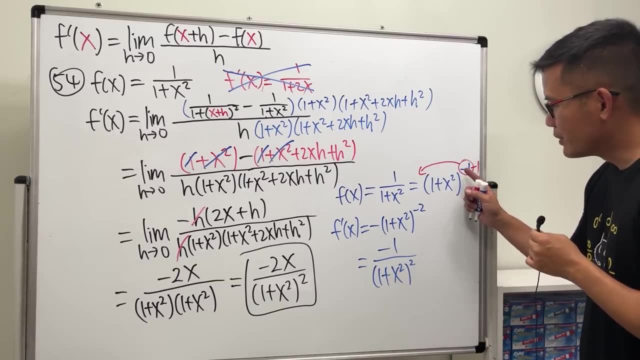 Definition is much better. Start it. So here's the deal. How can we come up with the 2x? Well, we're in calculus, So we have to think derivative. Here's the deal When we put the negative 1 to the front. 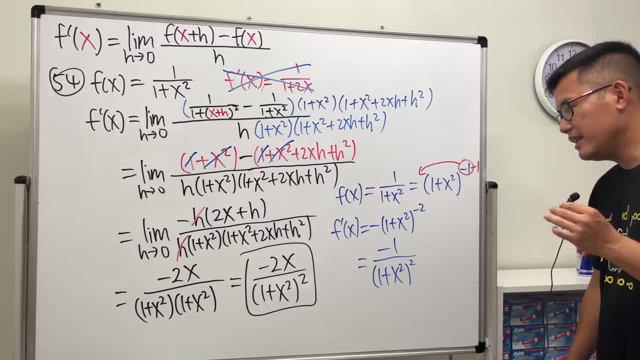 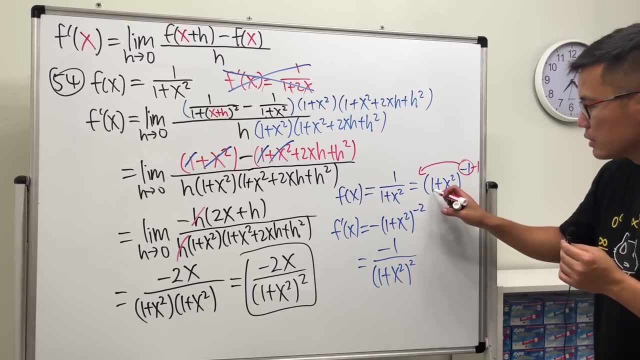 and then minus 1, we just do the power rule on the outside And the idea is you also have to look inside to see what the function is and multiply the derivative of that, So you see the derivative of this. The derivative of 1 is 0.. 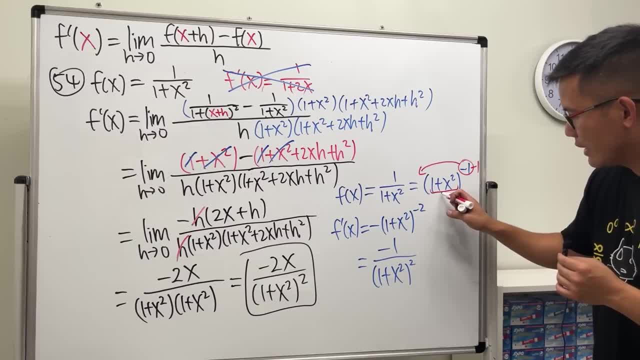 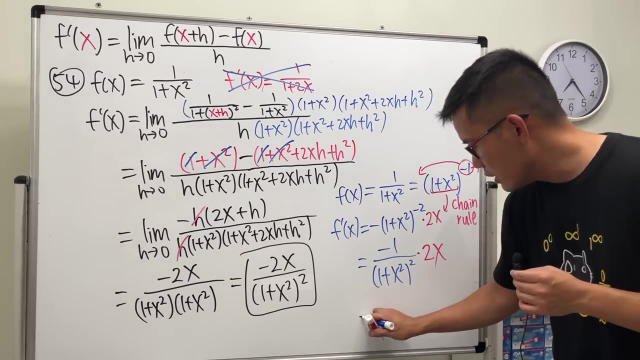 But the derivative of x squared is 2x. So we have to multiply this by 2x. So this is the so-called chain rule part Which is needed. So you see, if we multiply by 2x, all together we have: 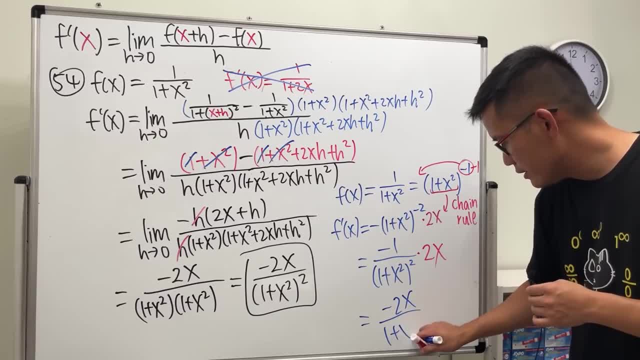 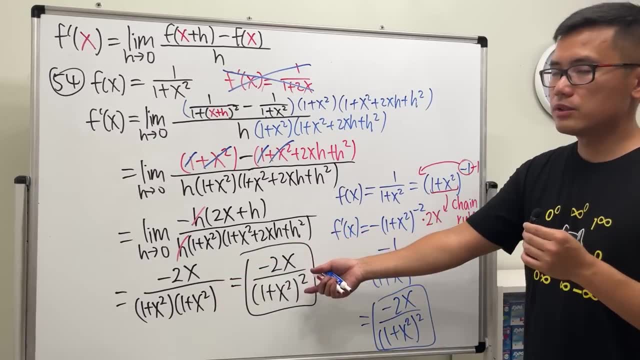 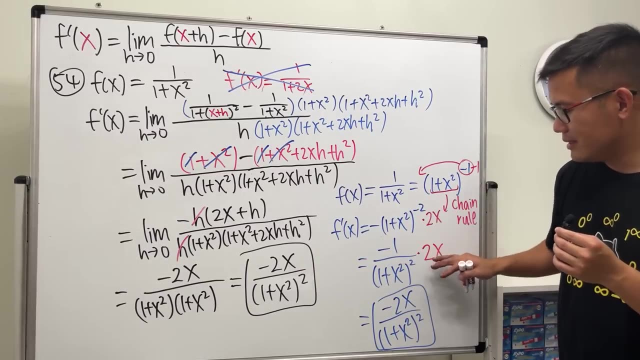 the answer that we have earlier. So hopefully you guys can see why we need the definition of derivative. It tells you what has to be right. If you want to use the shortcut well earlier without seeing that, then we'll miss the 2x. 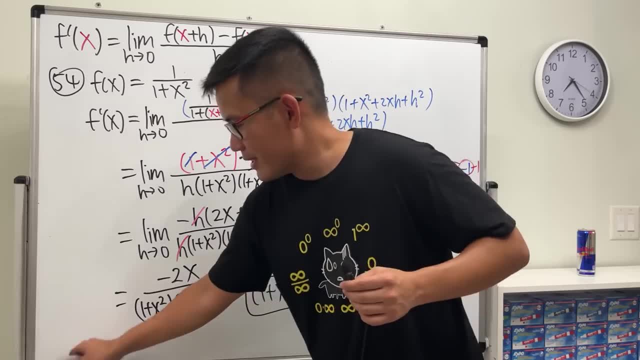 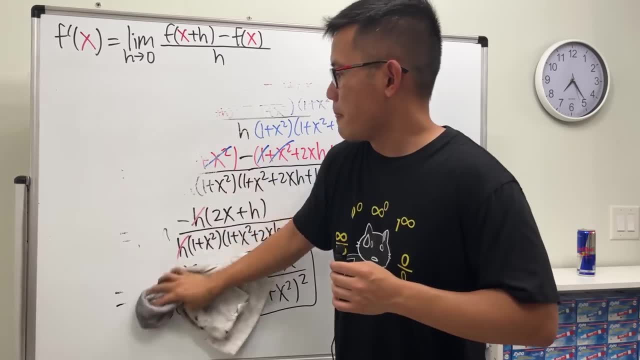 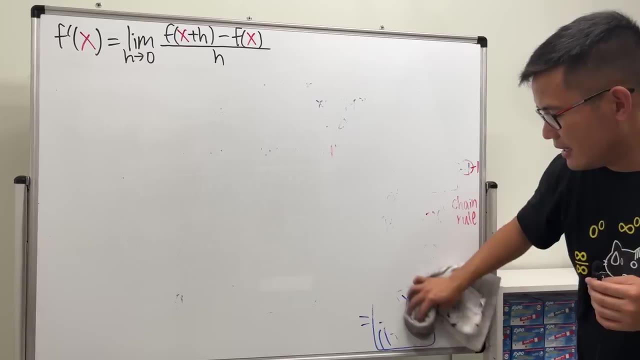 So that's the reason for the definition of derivative. And then let's do it again for number 55.. And maybe you guys can count how many times have I said: here's the deal. I don't know, I don't know why I kept saying: 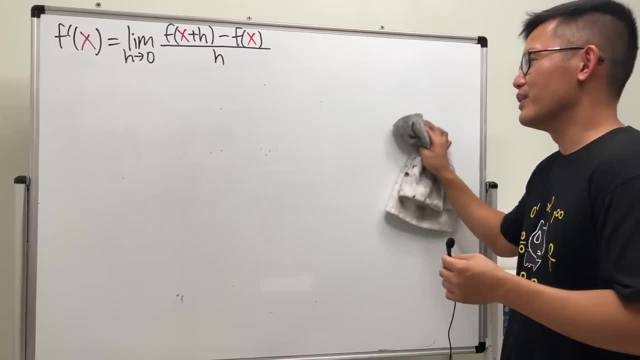 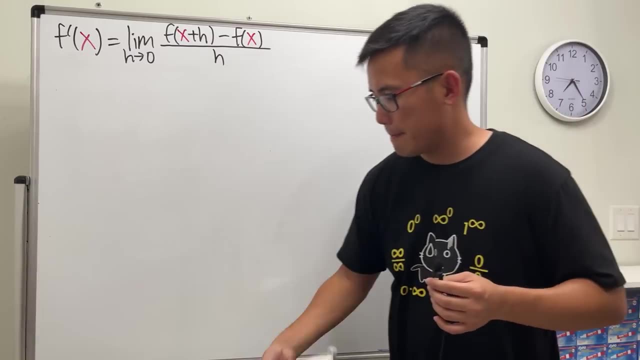 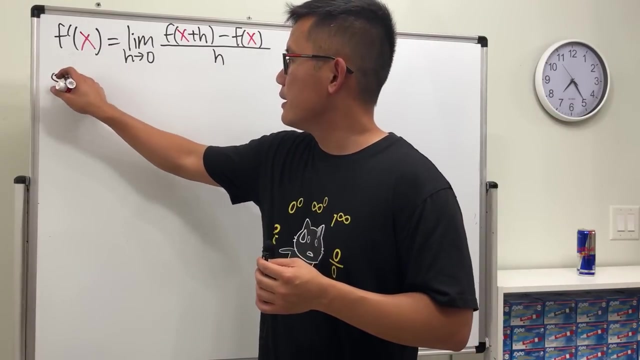 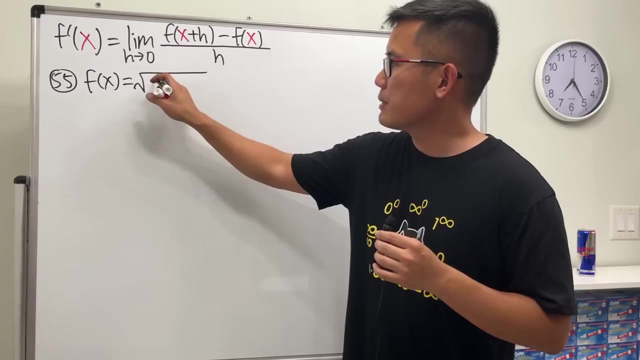 know, i don't know why i kept saying: here's the deal, here's the deal, especially for this video. i have no idea. number 55 f of x equals square root and we have 3x plus 1. wow, yes, we can use the definition of derivative and we can also use the. 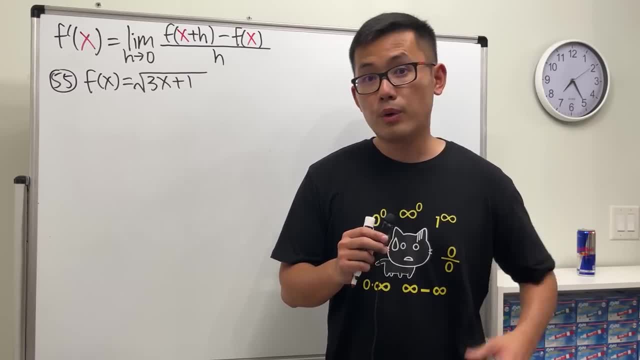 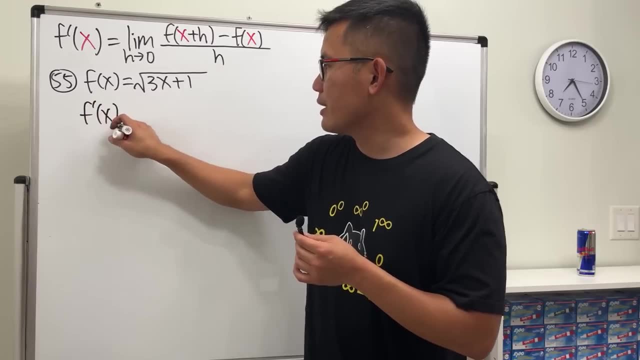 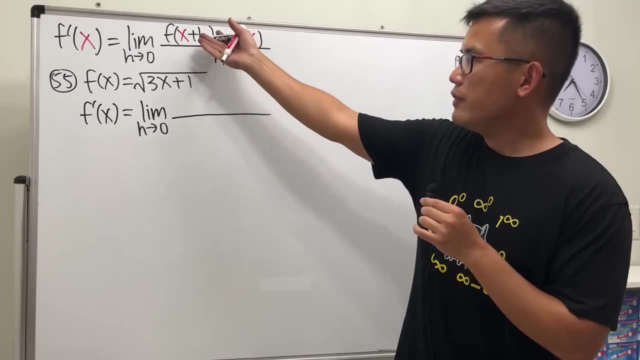 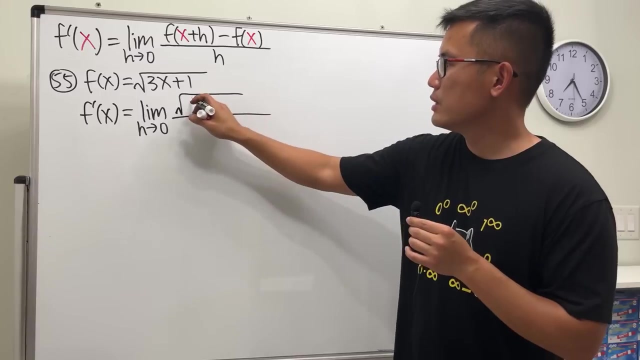 power rule and also the chain rule. you will see. first let's do the legitimate way, so all right, let's do it again. all right. f, prime of x equals the limit sh approaching zero. f of x plus h. you change the x to f, you change the x to x plus h, so you have the square root, three parentheses, x plus h, and then 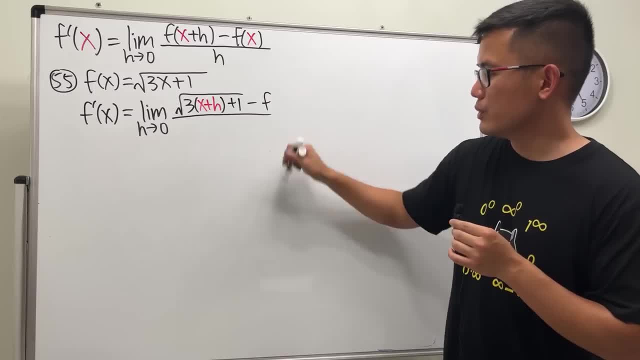 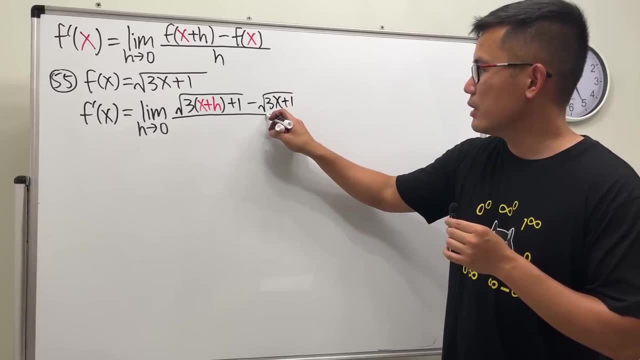 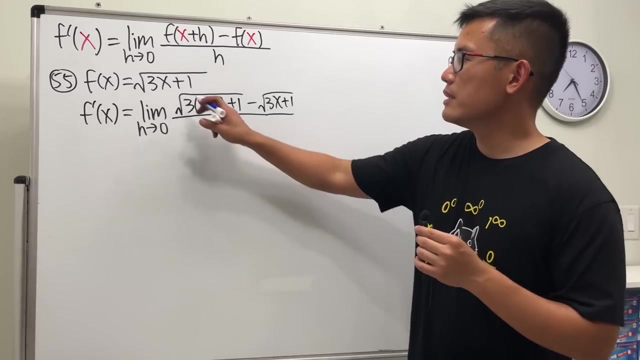 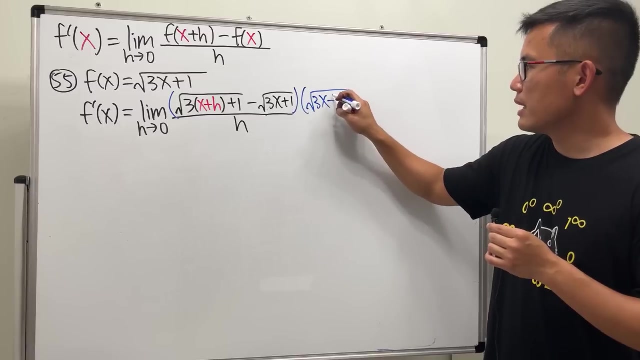 plus one and then minus the original function, which is just that. let's just just copy that down: square root of 3x plus h and then over h. okay, square root business, use the conjugate right. so let's multiply the top and bottom by square root and let's multiply this out so it's 3x plus. 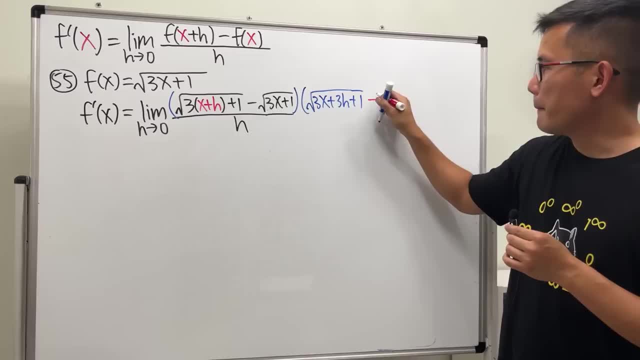 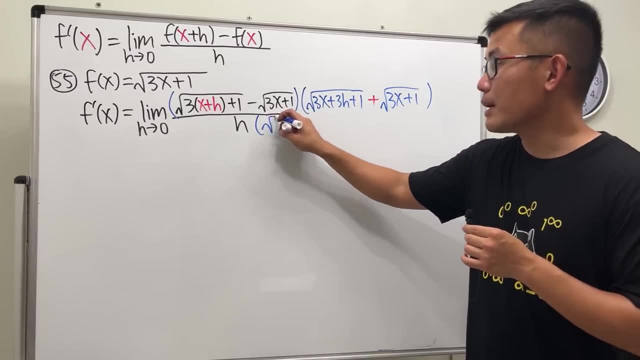 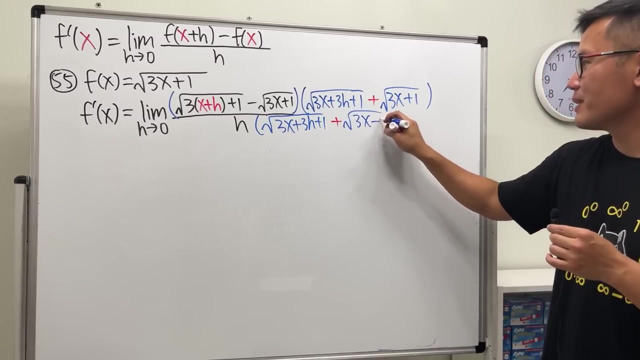 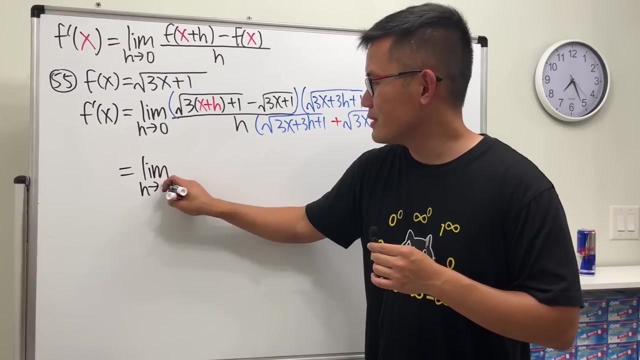 3h and then plus one, and then plus square root of that, which is 3x plus one. and let's do the on the top. on the bottom: 3x plus 3h plus one, plus square root of 3x plus one. cool, all right here. limit as h approaching zero. 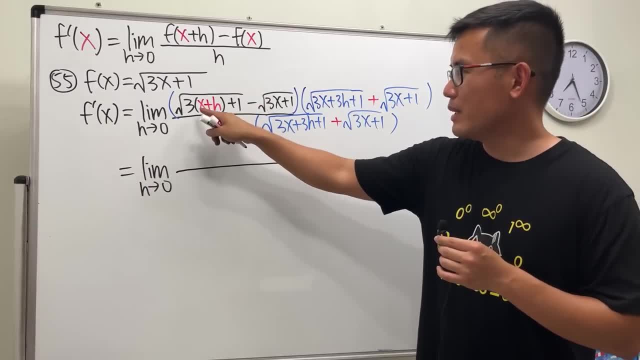 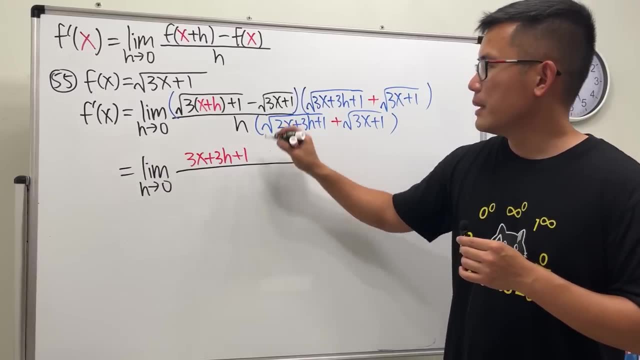 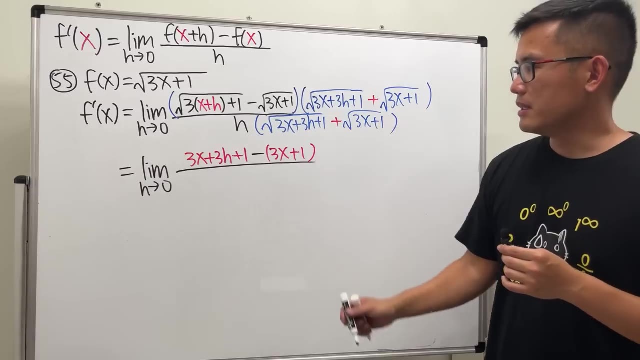 open the top right, multiply the top, we just get this square which is just inside here, 3x plus 3h plus one minus this thing square which is just 3x plus one you, and then the bottom stays the same. huh, so we have h times square root. 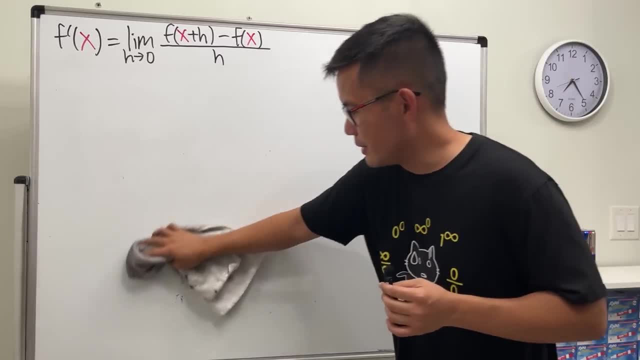 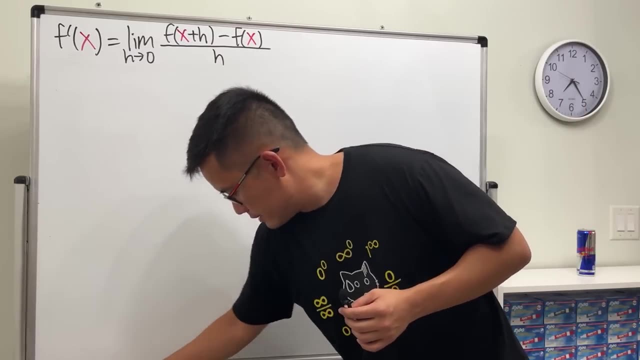 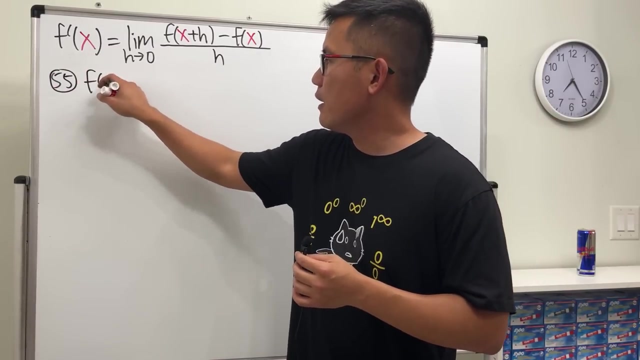 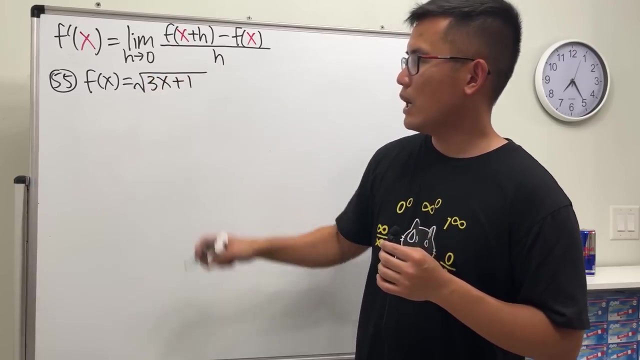 here's the deal. here's the deal, Especially for this video. I have no idea. Number 55.. f of x equals square root and we have 3x plus 1.. Wow, Yes, We can use the definition of derivative. 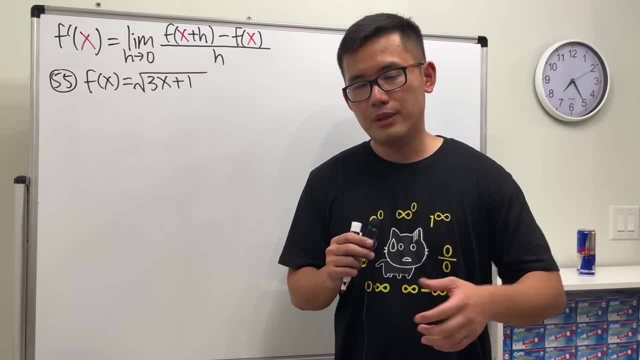 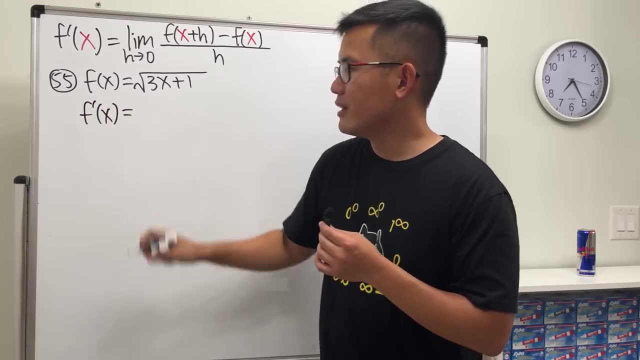 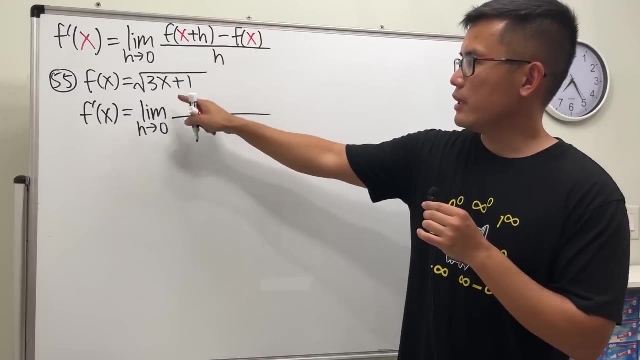 and we can also use the power rule and also the chain rule. You will see. First let's do the legitimate way. f prime of x equals the limit sh approaching 0. f of x plus h. you change the x to f. you change the x to x plus h. 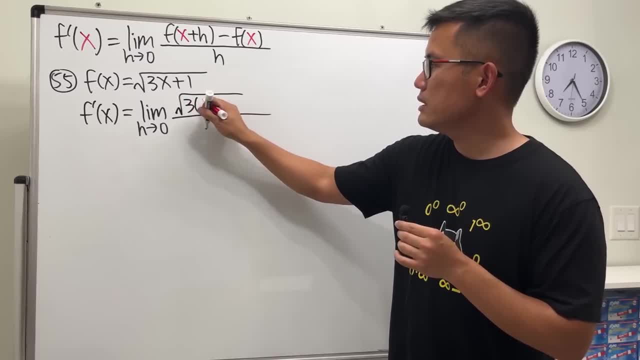 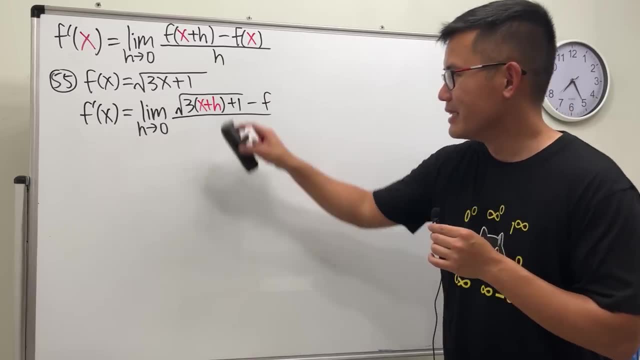 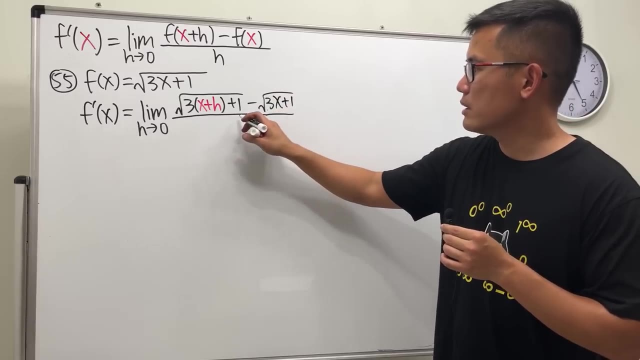 So you have the square root, 3 parentheses x plus h and then plus 1 and then minus the original function, which is just that. Let's just copy that down: Square root of 3x plus h and then all over h. Okay. 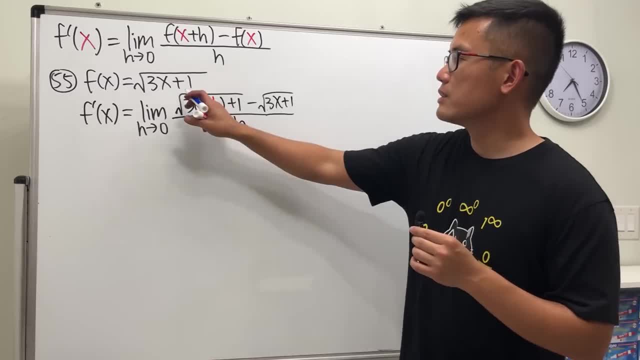 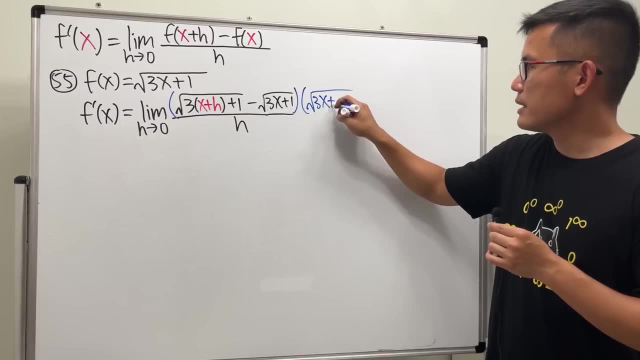 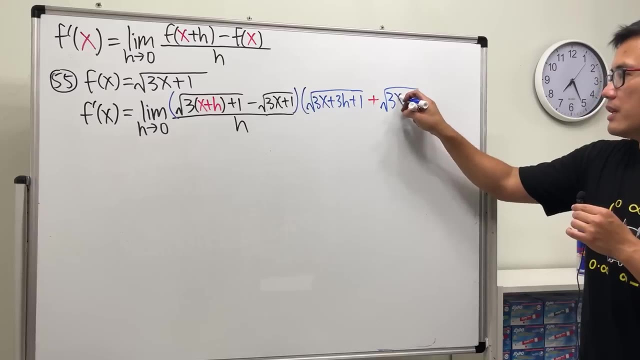 Square root business. use the count, you get right. So let's multiply the top and bottom by square root and let's multiply this out, So it's 3x plus 3h, and then plus 1, and then plus square root of that, which is 3x plus. 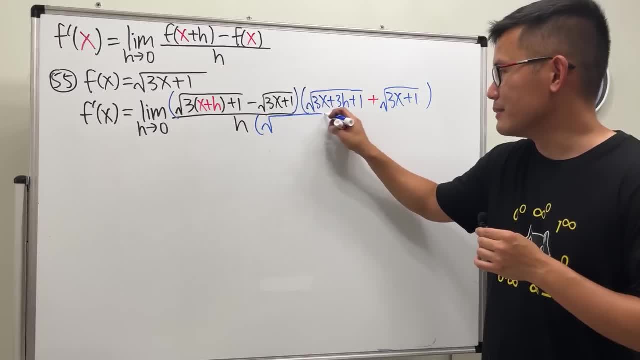 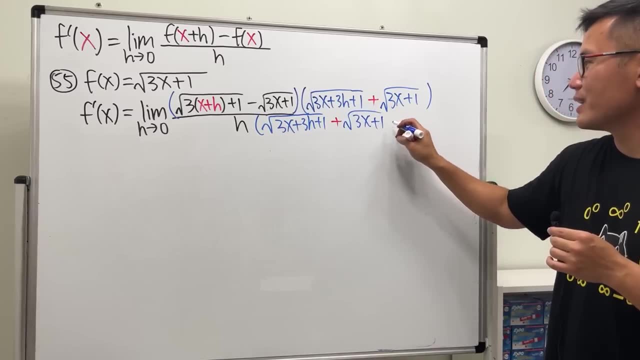 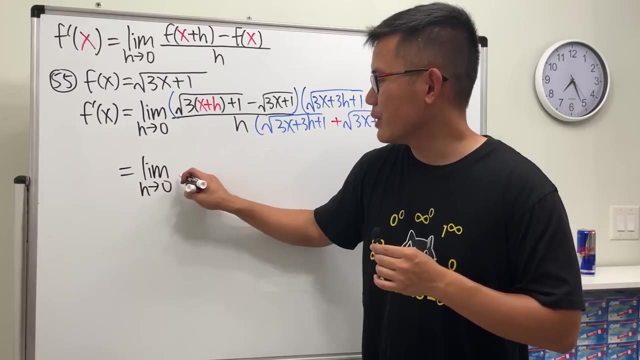 1. And let's do the same on the top. On the bottom, 3x plus 3h plus 1 plus square root of 3x plus 1.. Cool, Alright Here. Limit sh approaching 0, Open the top. 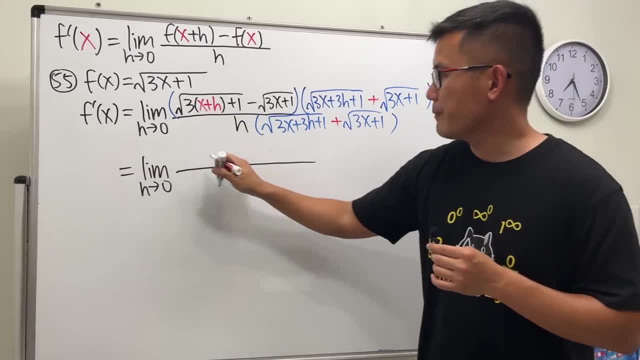 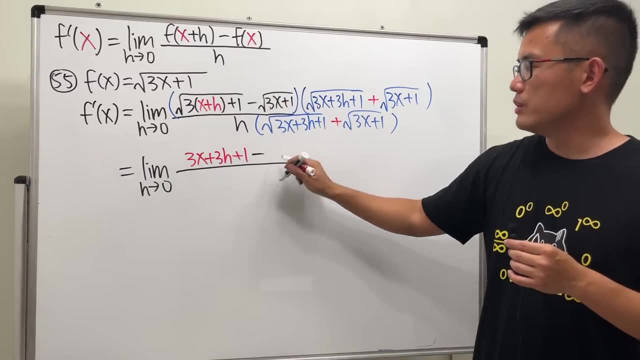 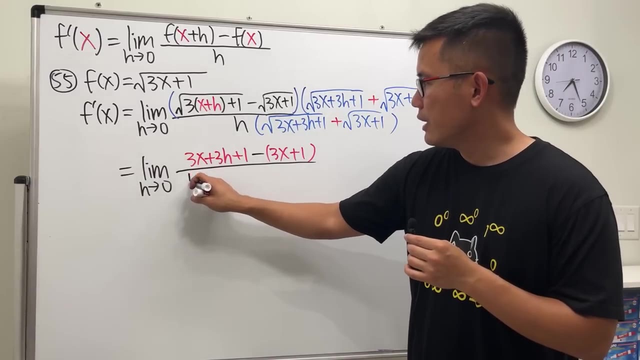 and multiply the top, We just get this square which is just inside here, 3x plus 3h plus 1.. minus this thing square which is just 3x plus 1. And then the bottom stays the same. So we have h. 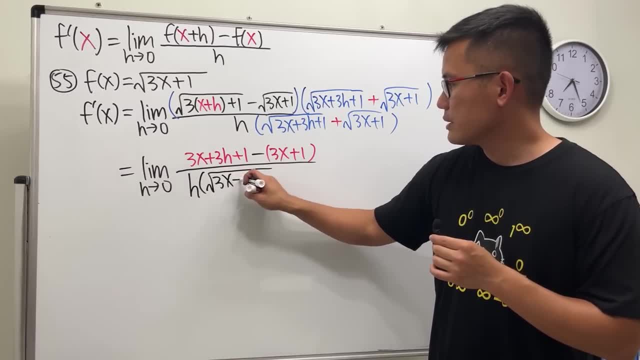 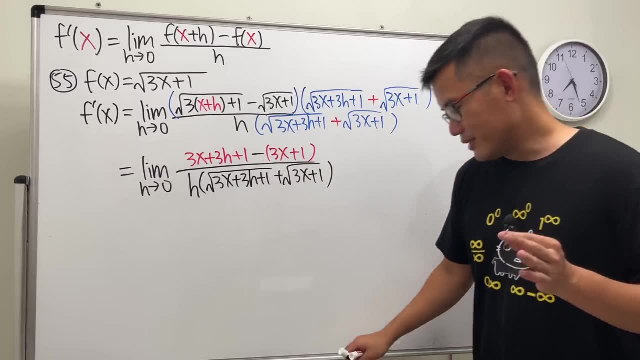 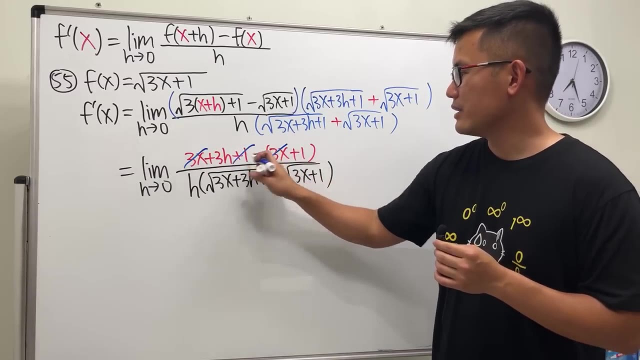 times square root, 3x plus 3h plus 1, and then plus square root of 3x plus 1.. Ladies and gentlemen, 3x minus 3x, this and that. cancel, 1 minus 1, cancel Perfect. On the top, we have 3 times h now. 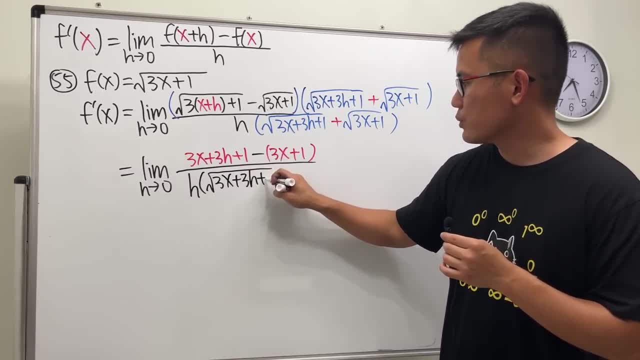 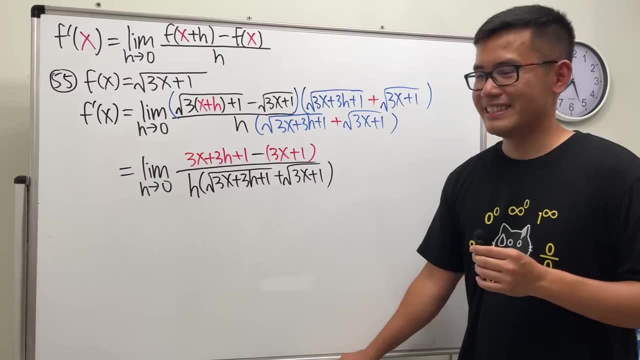 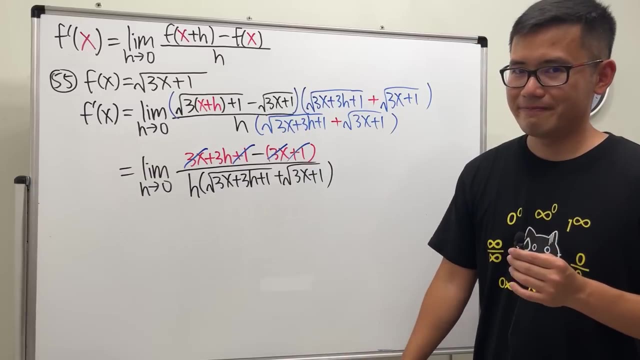 3x plus 3h plus one, and then plus square root of 3x plus one. ladies and gentlemen, 3x minus 3x, this and that. cancel. one minus one, cancel, perfect. on the top, we have three times h. now on the bottom, here, we have h times all that. so this h. 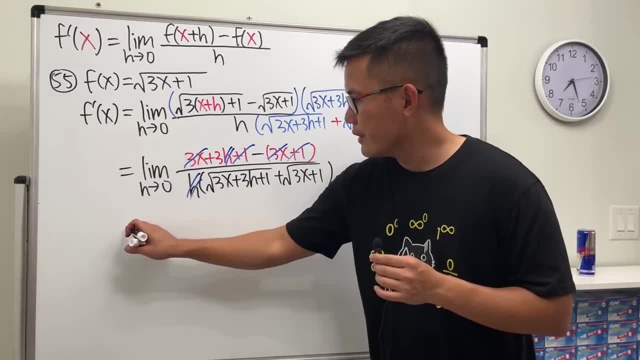 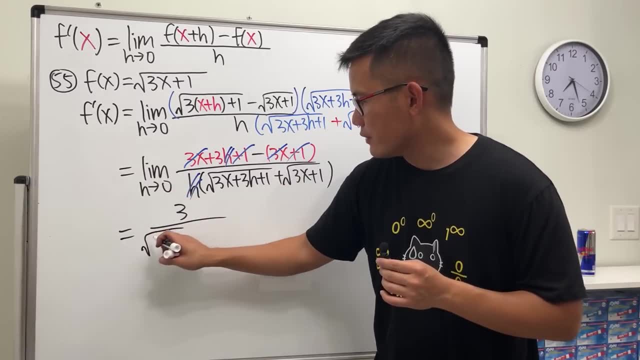 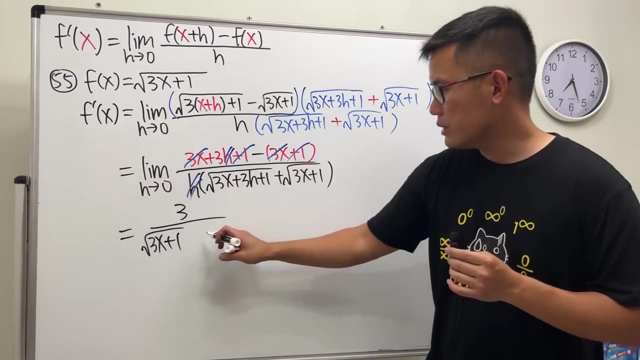 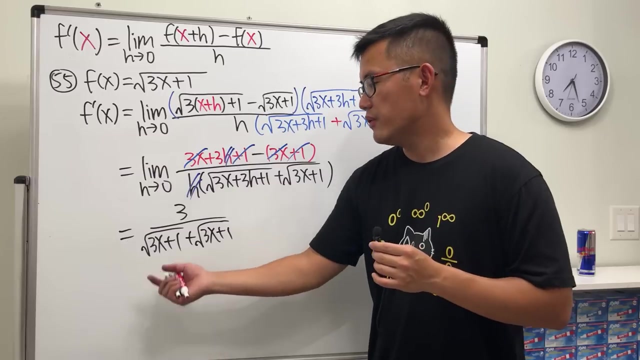 and that edge cancel. cool, therefore, we have a 3 on the top over. put 0 into here, so we have square root of 3x plus 1. that's the first square root, and now we actually have another one. huh, wow, and it happened to be the same and we're adding: therefore it becomes two of them. so on all. 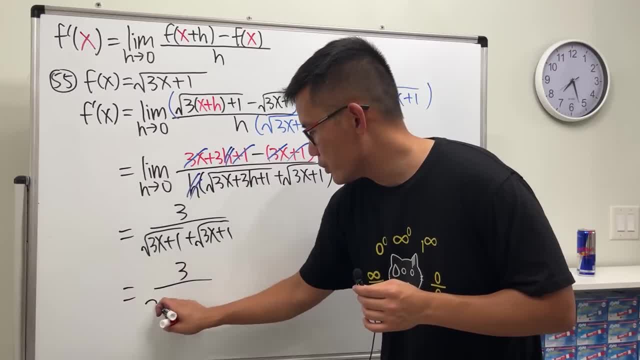 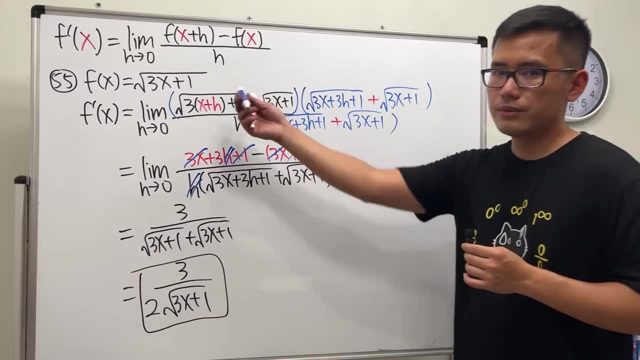 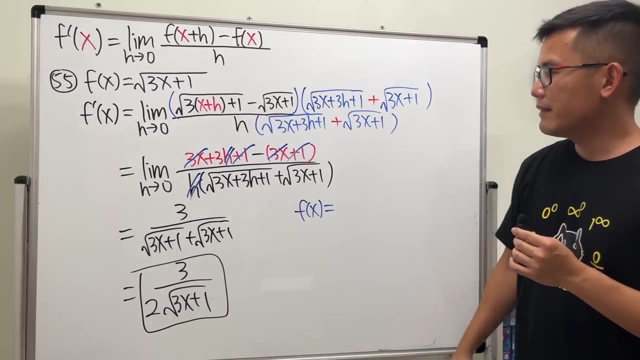 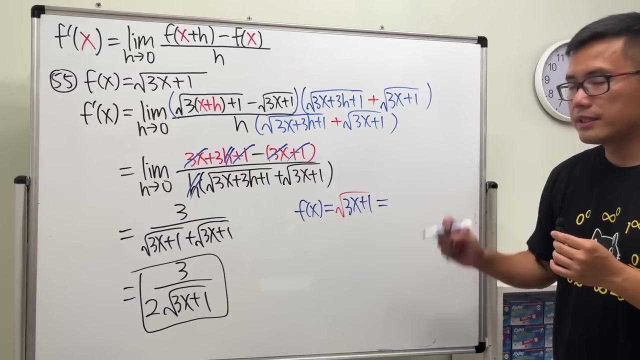 we have 3 over 2. square root of 3x plus 1 done now, the moment that you have been waiting for. f of x equals okay, we have the square root of 3x plus 1, but, as i said earlier, let's write the square root as 1 half power. that way we can use the power rule. 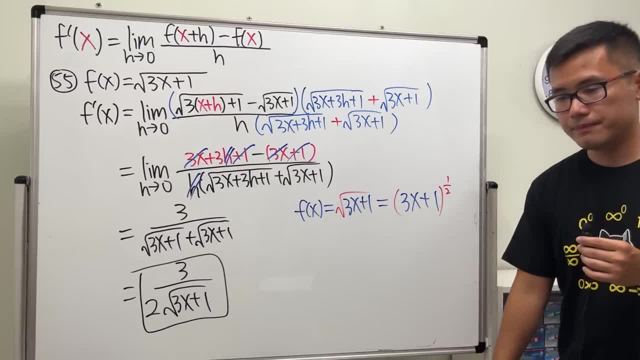 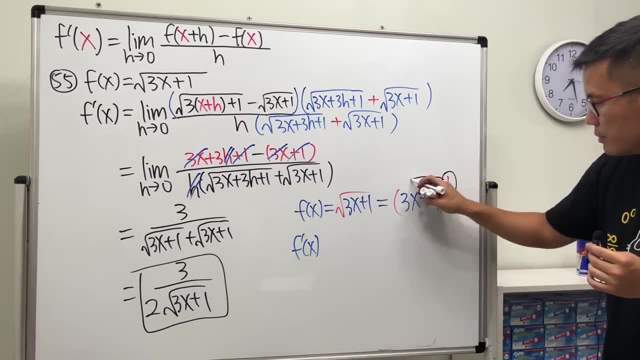 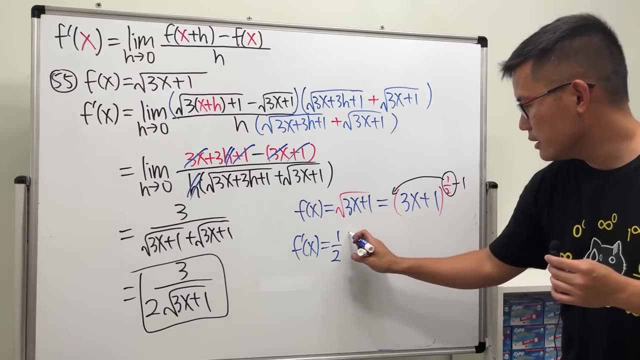 so 3x plus 1 raised to the 1 half power. once we do this, we can go ahead and use the power rule, meaning that put the power to the front minus 1, so we have the 1 half at the front and then the inside is 3x plus 1. 1 half minus 1 is negative 1 half. 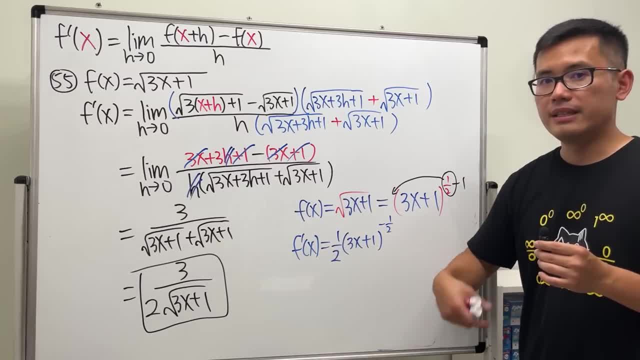 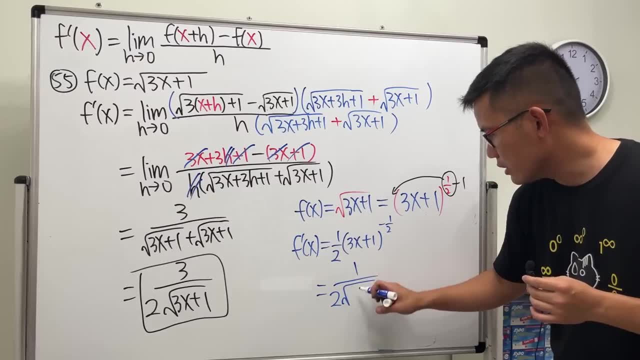 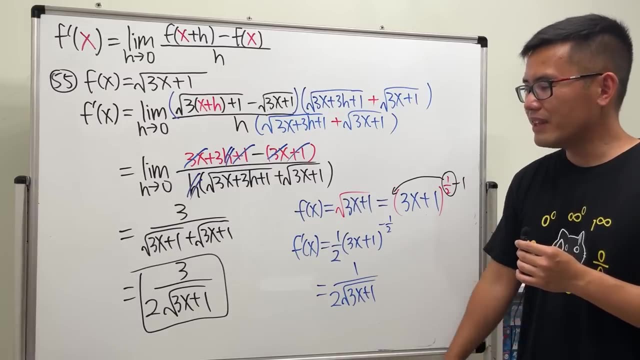 negative. 1 half is the same as bring this down to the bottom and then give it a square root to it. so we have 1 over 2, square root of 3x plus 1. ah, man, this is what we have now. that's what we got earlier. 3 on the top. 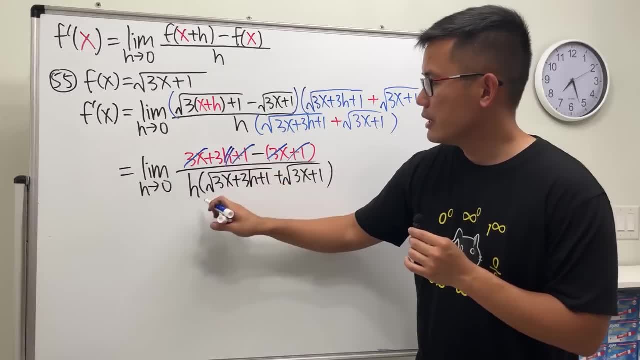 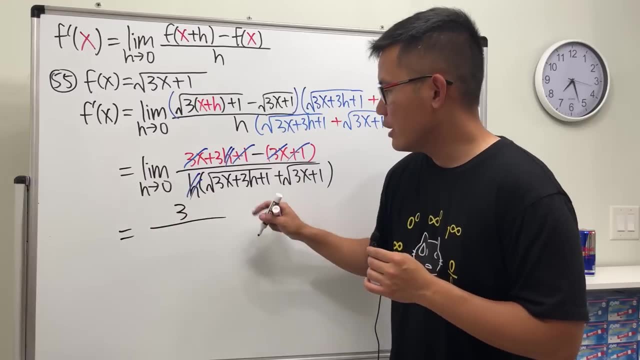 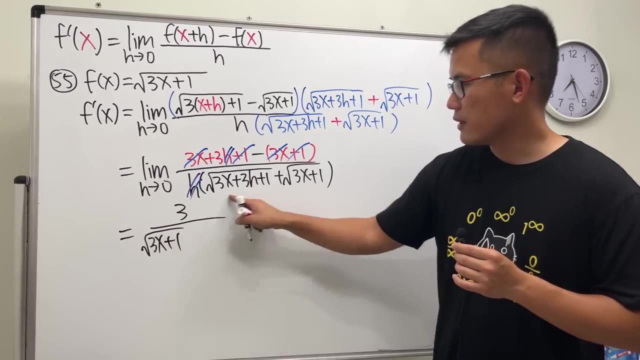 On the bottom here we have h times all that. So this h and that h cancel Cool. Therefore we have 3 on the top over. put 0 into here, So we have square root of 3x plus 1. That's the first. 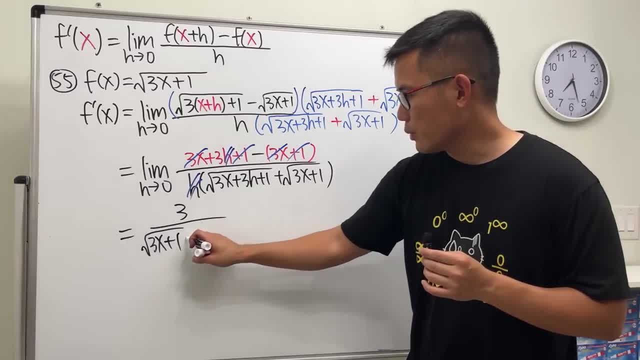 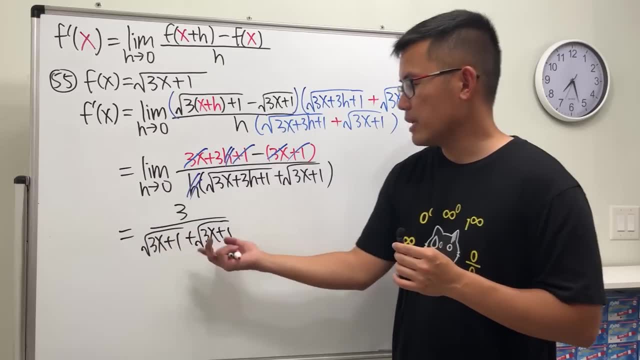 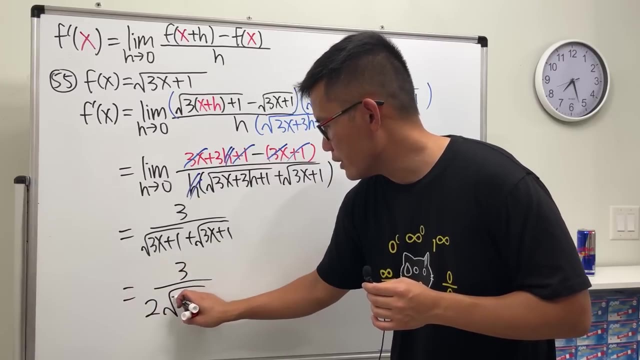 square root And we actually have another one. Wow, And it happened to be the same And we're adding. Therefore it becomes 2 of them. So all in all, we have 3 over 2 square root of 3x plus 1.. 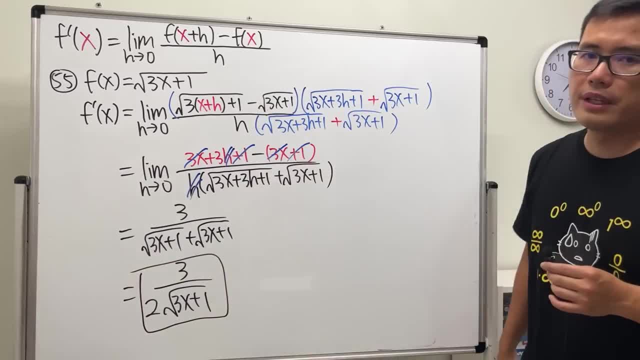 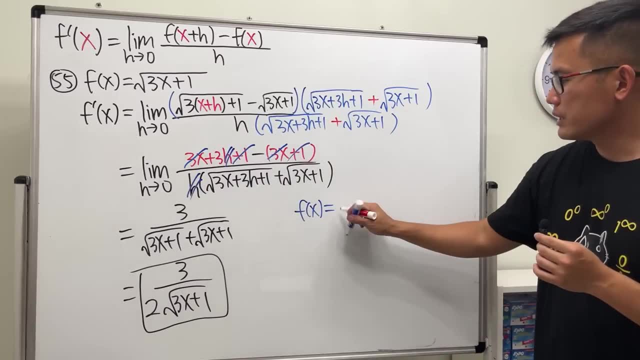 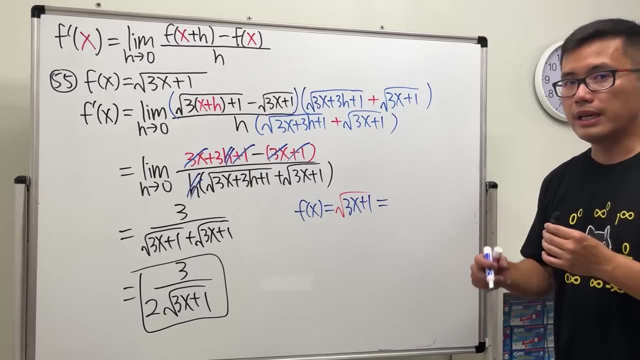 Done Now, the moment that you have been waiting for. f of x equals. okay, we have the square root of 3x plus 1.. But, as I said earlier, let's write the square root as 1 half power. We can use the power rule. 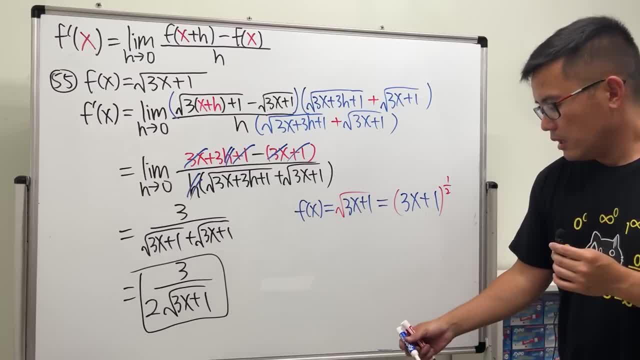 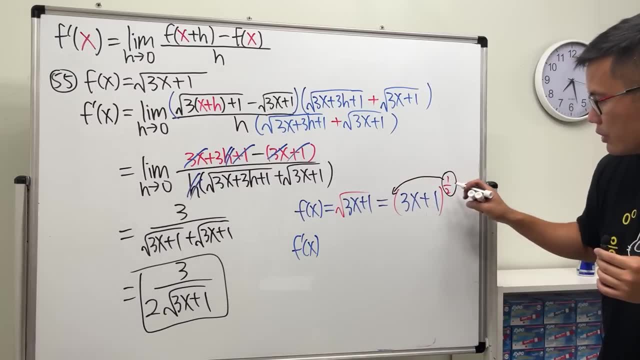 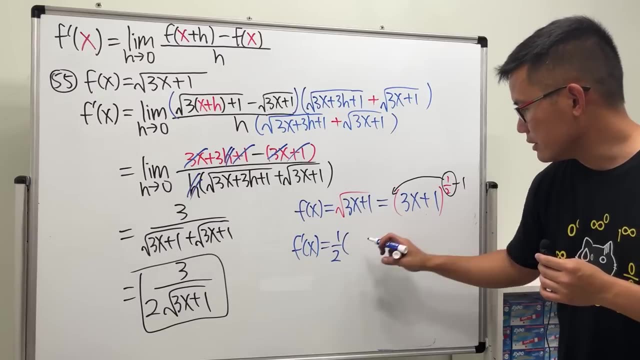 So 3x plus 1 raised to the 1 half power. Once we do this, we can go ahead and use the power rule, Meaning that put the power to the front minus 1, so we have the 1 half at the front and then. 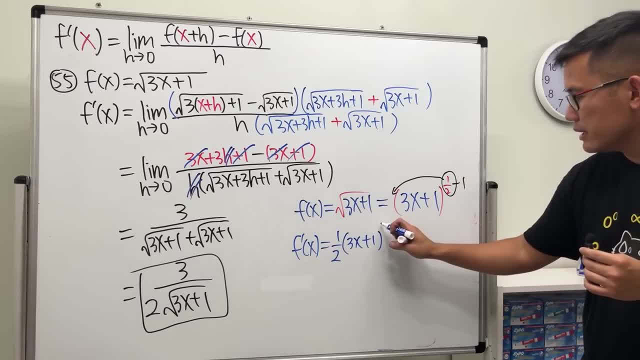 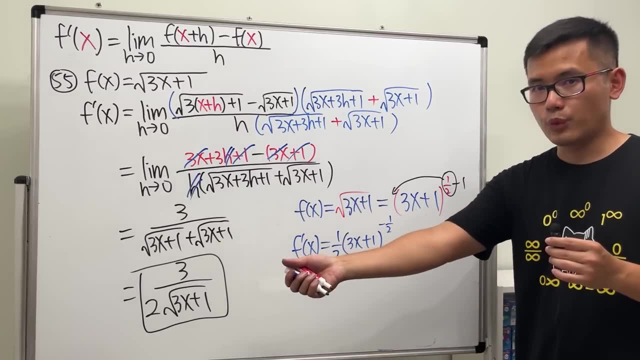 the inside is 3x plus 1. 1 half minus 1 is negative. 1 half Negative. 1 half is the same as bring this down to the bottom and give it a square root to it. So we have 1 over 2. 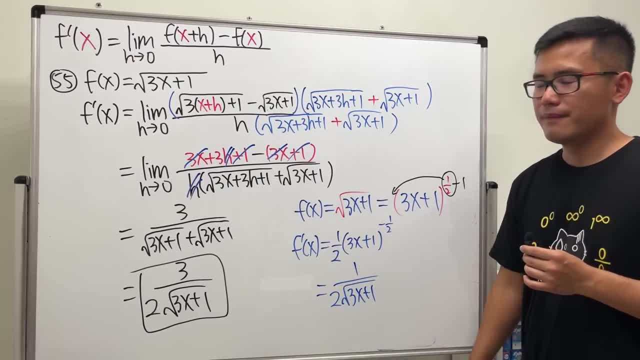 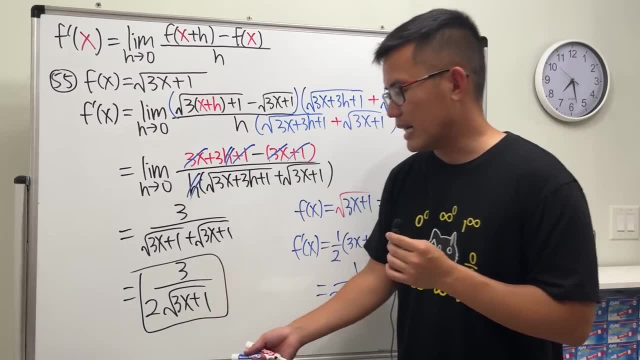 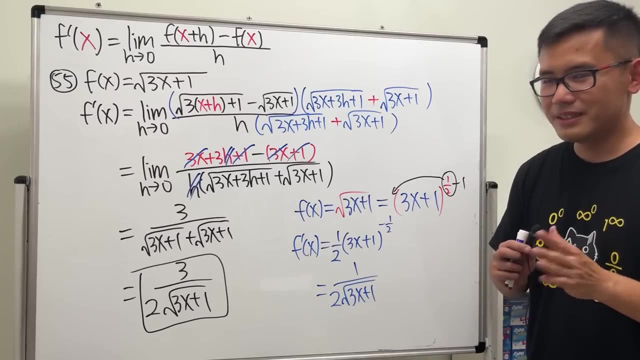 square root of 3x plus 1.. Ah man, This is what we have now. That's what we got earlier. 3 on the top, We only have 1.. Where are the other 2?? 1 plus 3.. 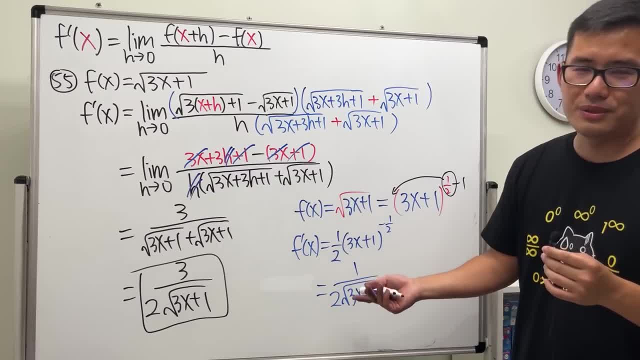 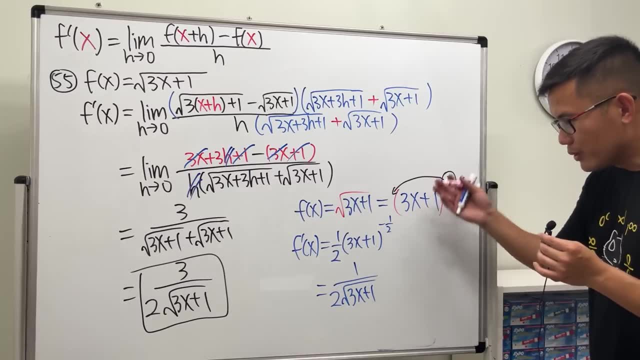 we all have a 1. where are the other two? 1 plus 3? 1 plus 2 is 3. not funny, i know, but you know the deal. what you will have to do when you're doing this process is that once you do the power rule on the 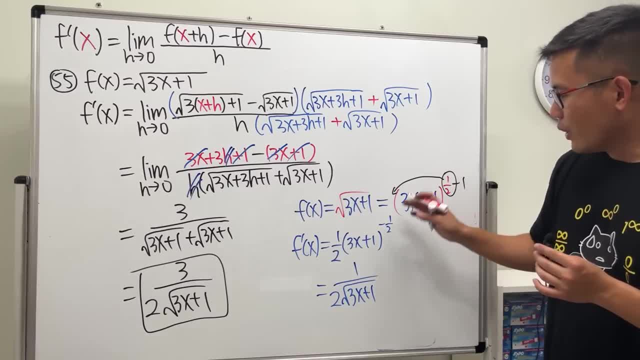 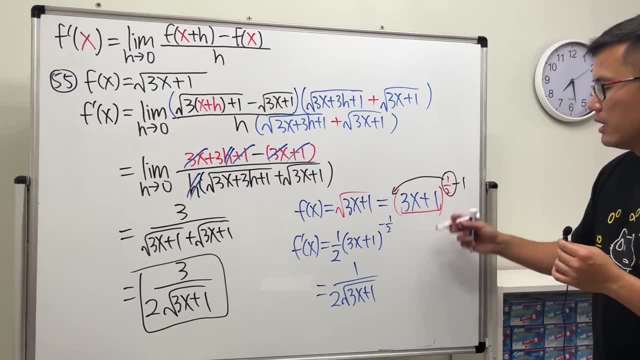 Not funny, I know, But you know the deal. What you will have to do when you are doing this is that, once you do the power rule on the outside, you will have to look at the inside and ask yourself: what's the derivative of the inside function? 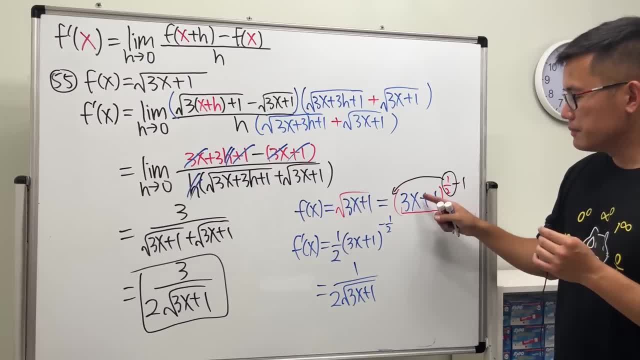 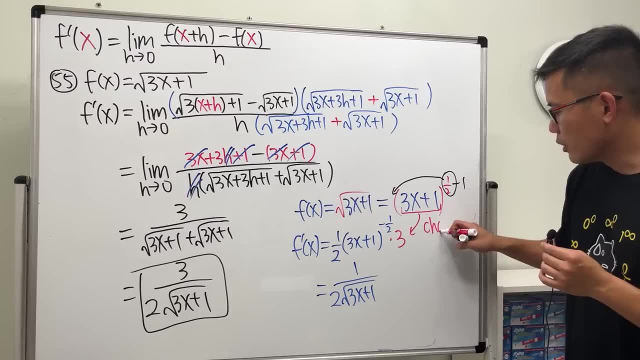 The derivative of 3x plus 1 is just a 3, right. So you will have to use the power rule inside again. So you have to multiply by 3.. Again, this part is the so called the chain rule part. And for more, 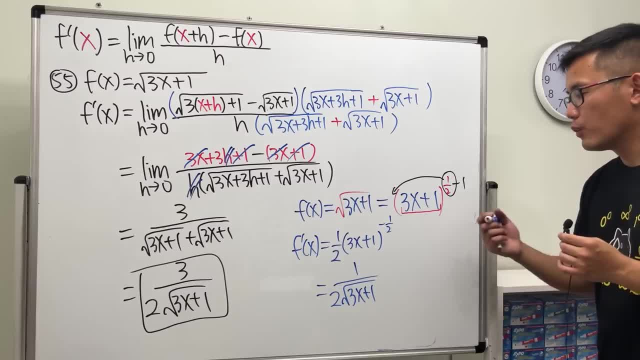 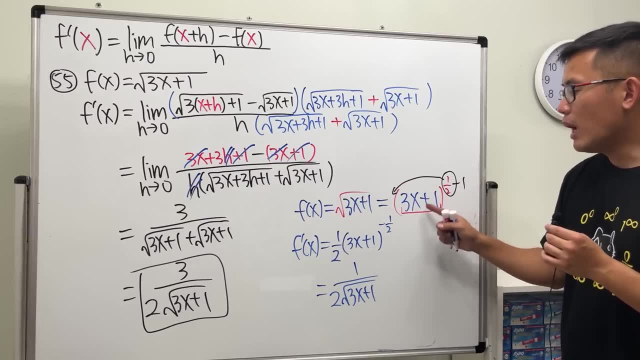 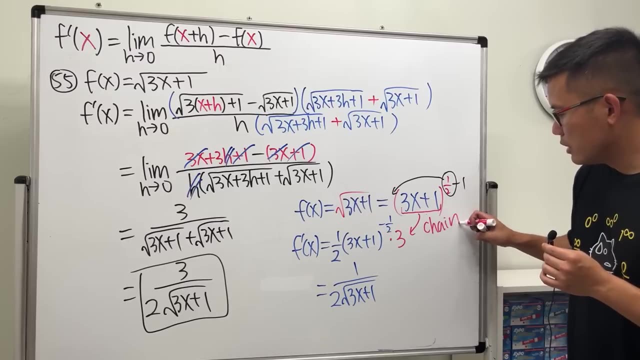 outside, you will have to look at the inside and ask yourself what's the derivative of the inside function? the derivative of 3x plus 1 is just a 3 right. so you will have to use the power rule inside again. so you have to multiply by 3 again. this part is the so-called the chain rule part, and 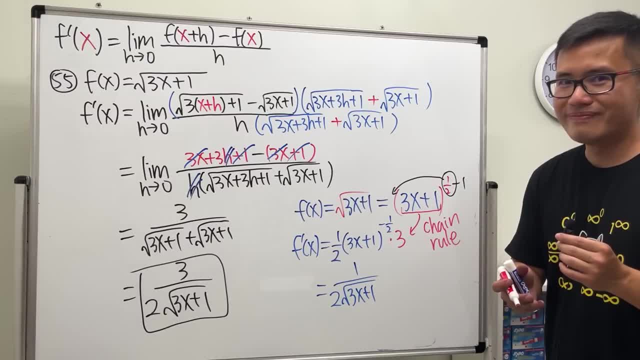 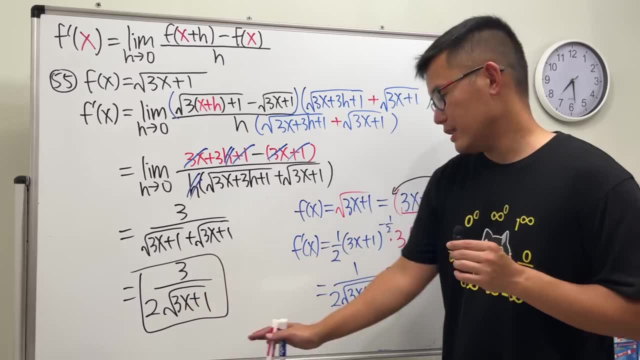 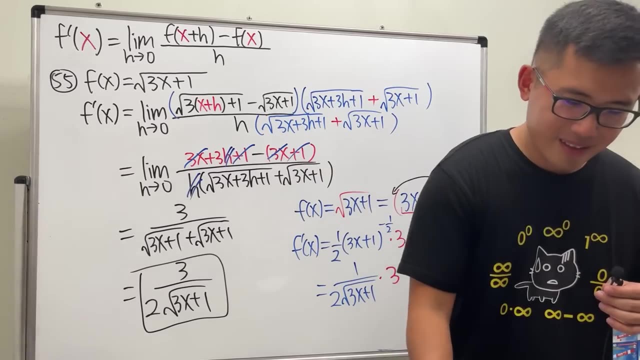 for more practice with derivative. you know where to go: 100 derivatives. so multiply by 3, multiply by 3 and we get that all right. so that's that, yay, done with the page five. now you think we're done with derivative. no, we can never run away from derivative. 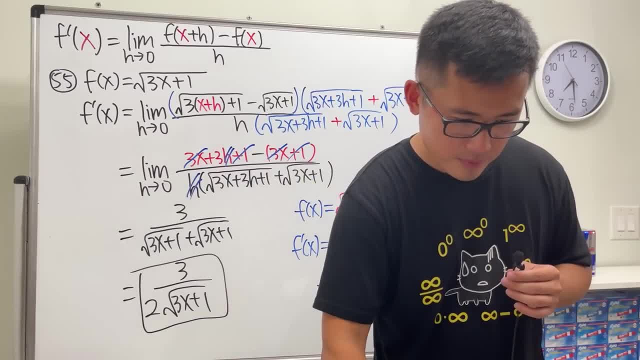 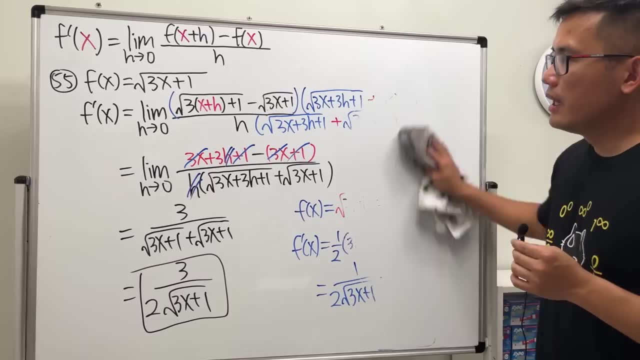 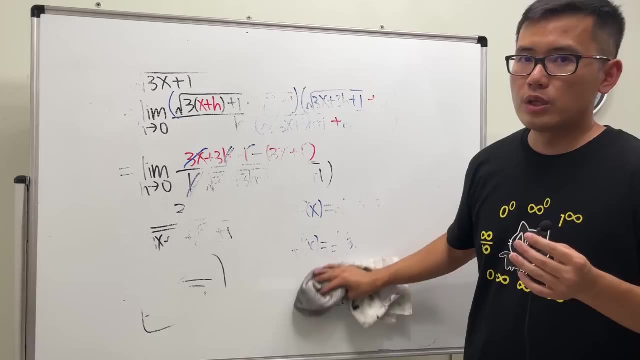 we have the lapidos rule and let's see, i'm going to give you guys a quick, quick, quick explanation on what the lobby toss rule is. and then, if you haven't studied derivative yet, then a lot of this wouldn't make sense, like: what's the derivative of natural log of x? what's the? 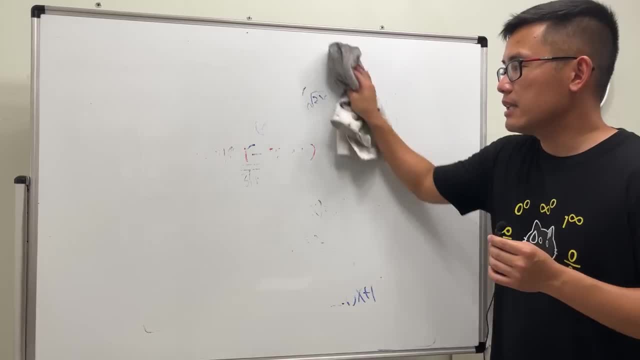 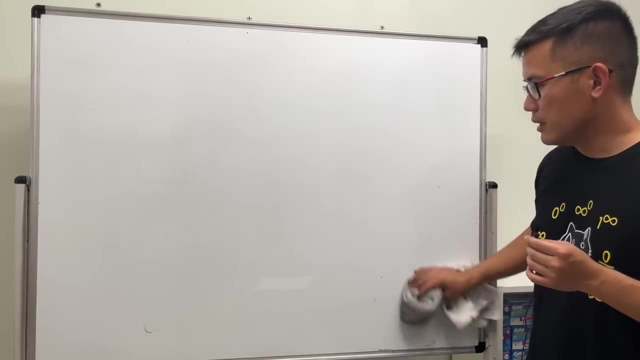 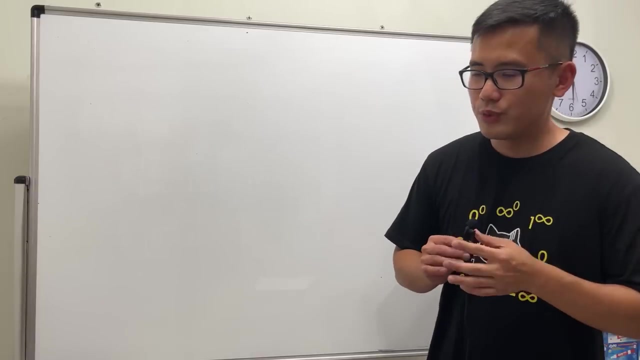 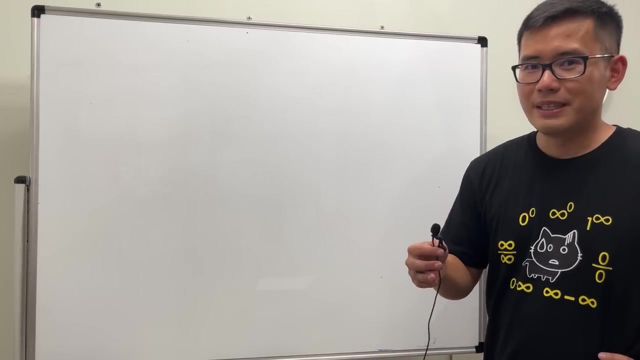 derivative of tangent x or things like that. so be sure you watch my other video for the derivatives. all right, maybe, uh, you're just taking cal 1, maybe like the first three weeks or so. this is like a good place for you to uh, maybe just stop and then later on. yeah, you can just stop and then later on you can. 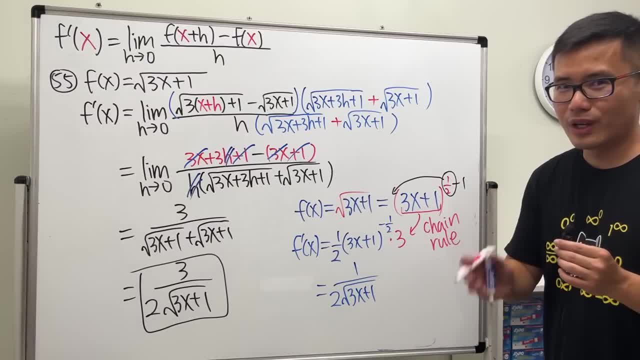 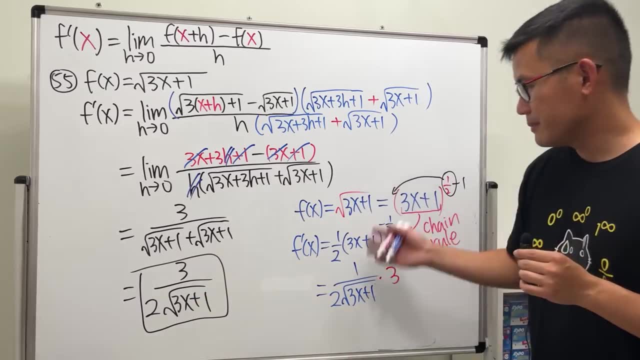 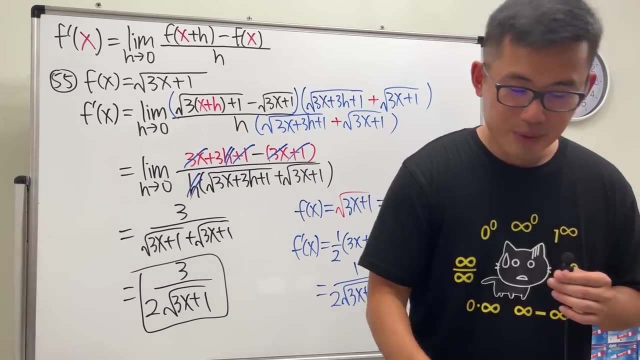 practice with derivative. you know where to go: 100 derivatives. So multiply by 3,, multiply by 3 and we get that Alright. so that's that, Yay, Done with the page 5.. Now you think we are done with. 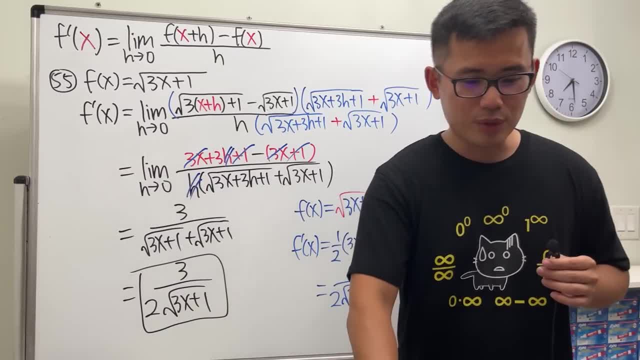 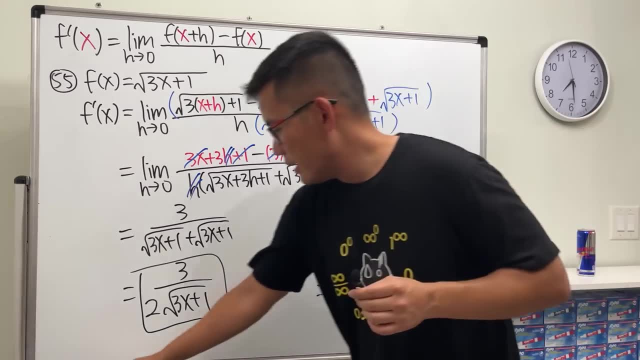 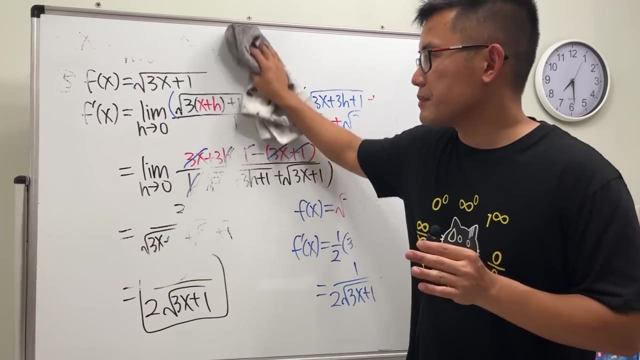 derivative. No, We can never run away from derivative. We have the Lapithos rule And let's see, I'm going to give you guys a quick, quick, quick explanation on what the Lapithos rule is and then, if you haven't, 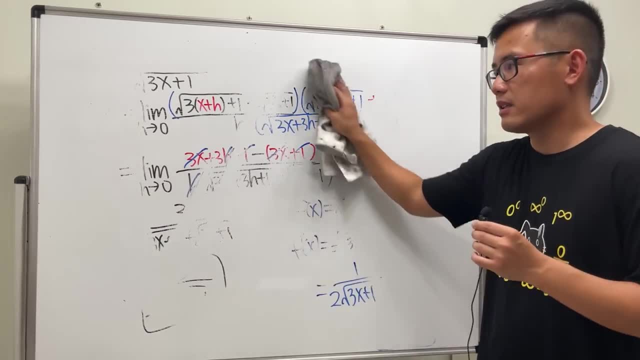 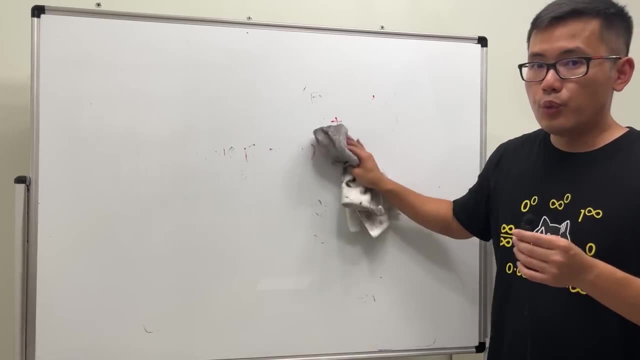 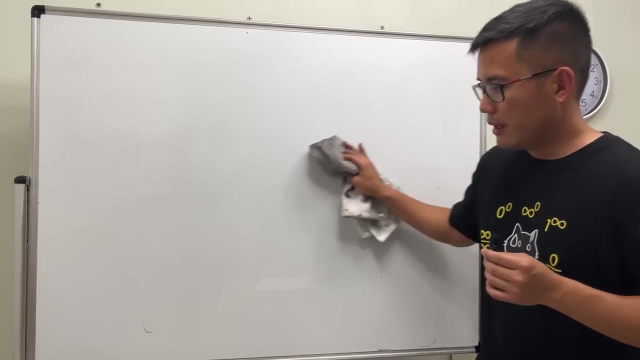 studied derivative. yet then a lot of this wouldn't make sense, Like what's the derivative of natural log of x, What's the derivative of tangent x, Or things like that. So be sure you watch my other video for the derivatives. Alright. 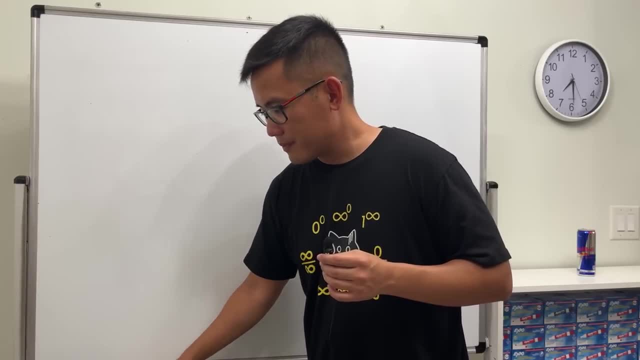 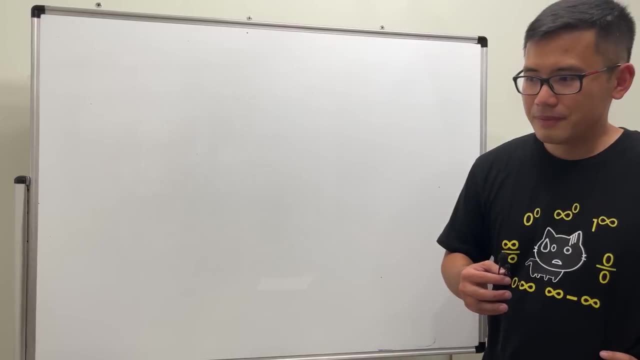 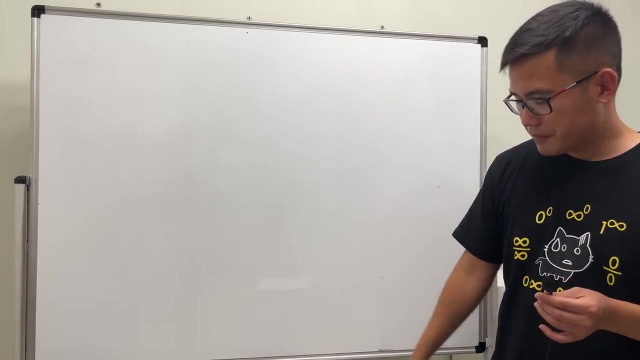 Maybe you are just taking Cal 1, maybe like the first 3 weeks or so. this is like a good place for you to maybe just stop and then later on you come back, starting at 56.. So usually question 1 to question 55 is like. 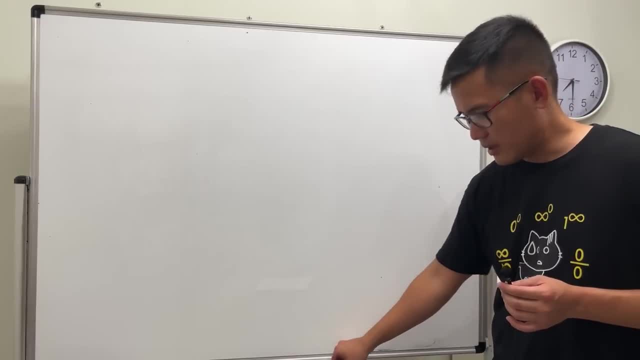 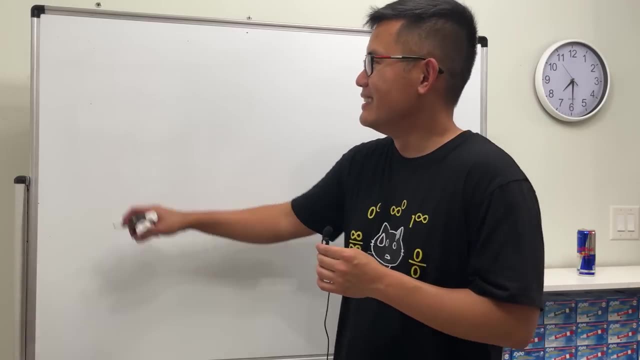 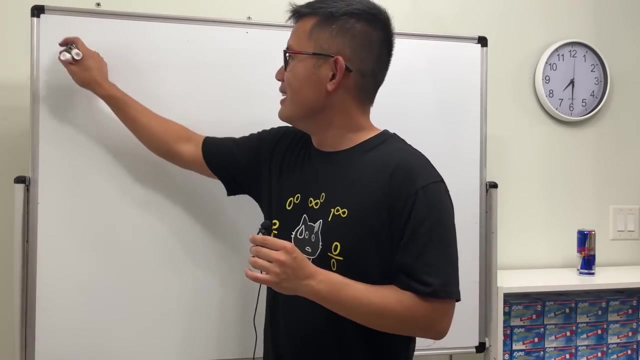 the first months for your Cal 1 class, Like first 3-4 weeks. Okay, I talk too much. No, no, no, no, no, I did 55 already. No, Ladies and gentlemen, let's have a look This time we want. 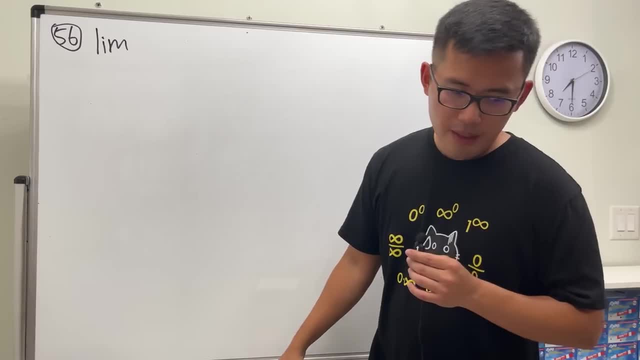 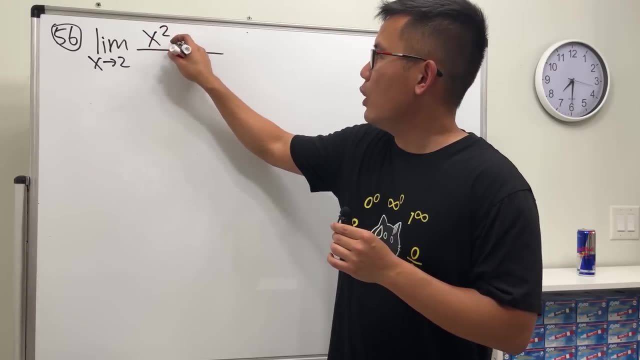 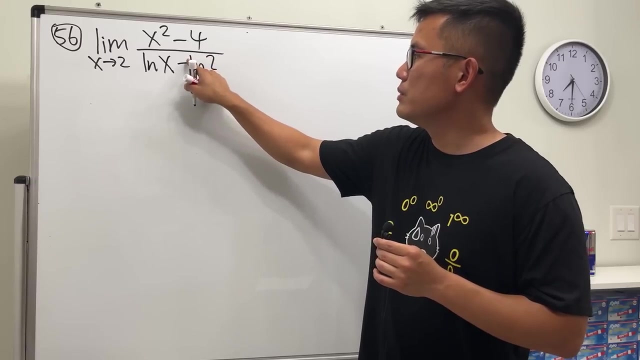 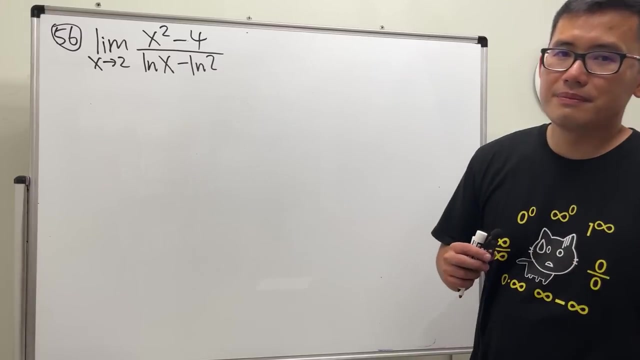 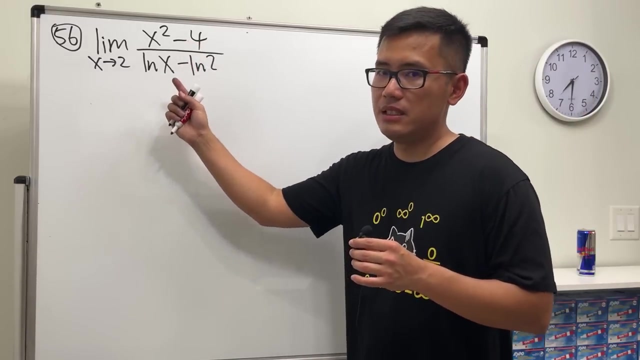 the limit, and we just want the limit as x approaching 2 and we have x squared over x squared minus 4 over ln, x minus ln 2. How do we do this? Factor it? Sure, We can factor the top easily, but how can we factor the bottom? 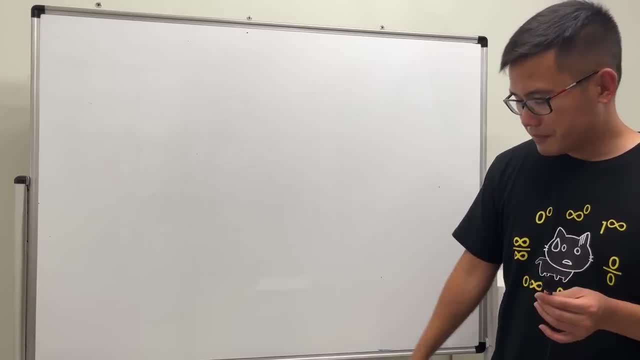 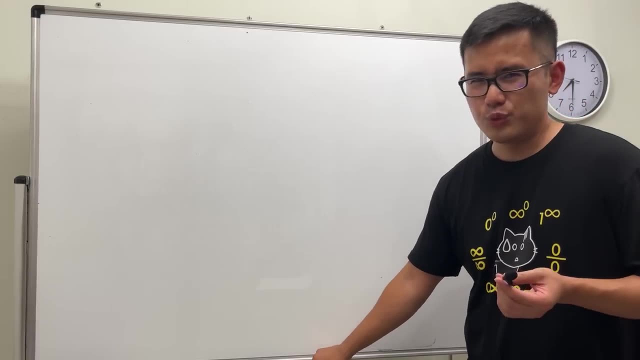 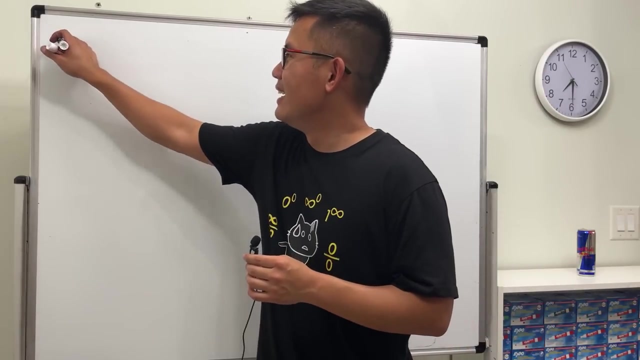 come back starting at 56.. so usually the question one to question 55 is: like the first months was when you cut one class, like first three, four weeks. okay, i talk too much. no, no, no, no, i did 55 already. no, ladies and gentlemen, let's have a look. this time we want. 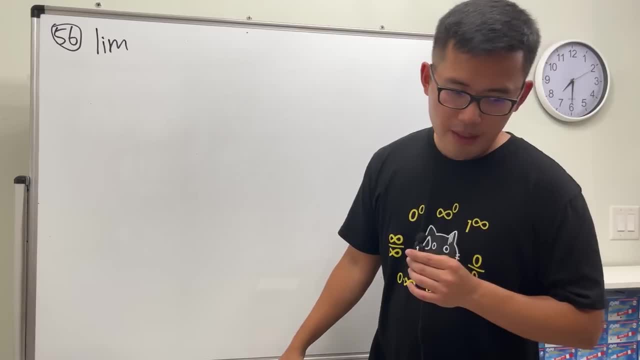 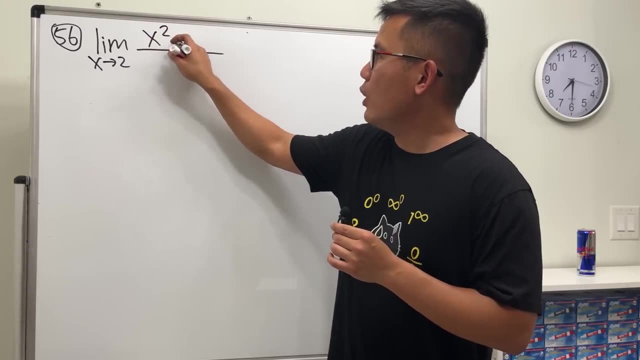 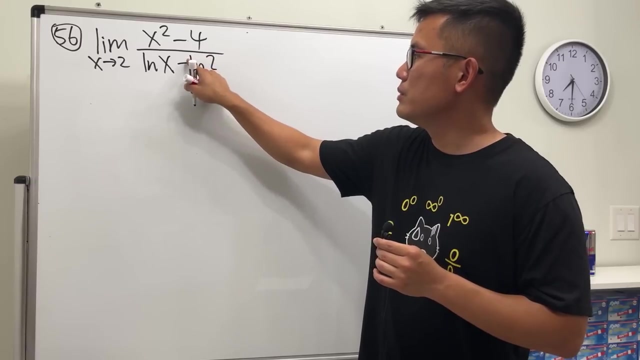 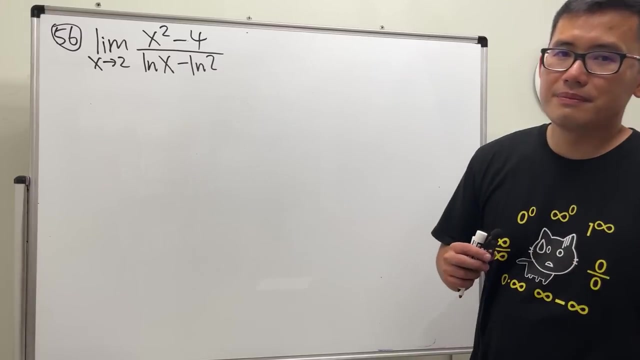 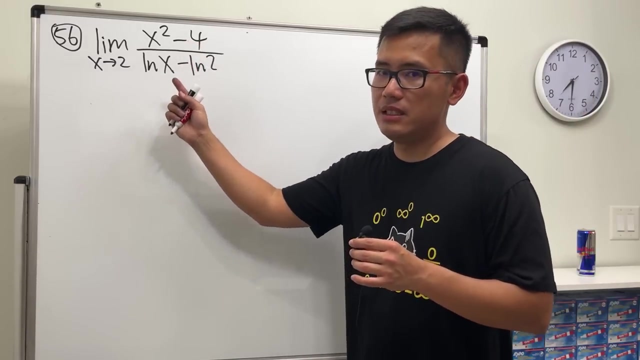 the limit, and we just want the limit as x approaching 2 and we have x square over, so x minus x, squared minus 4 over ln, x minus ln 2. how do we do this factor? it sure can factor the top easily, but how can we factor the bottom, ln x minus ln 2.. Is this? 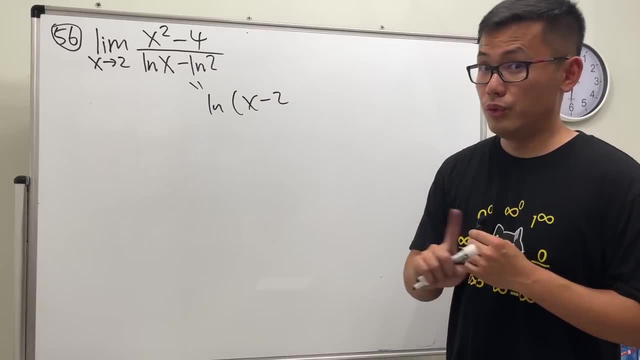 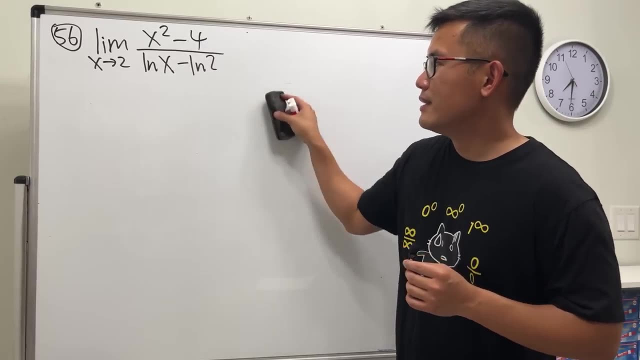 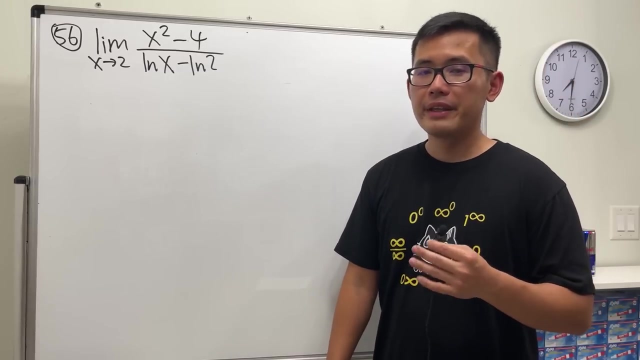 just the same as ln, and then x minus 2? No, no, don't do that. It's not ln time, Don't? no? This is not even funny. No, don't do that. No, Wow, So here is the time that I'll show. 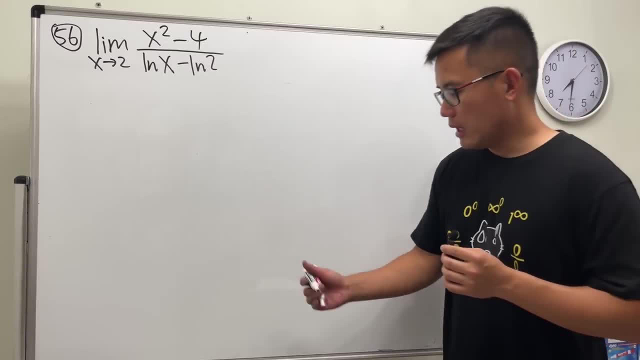 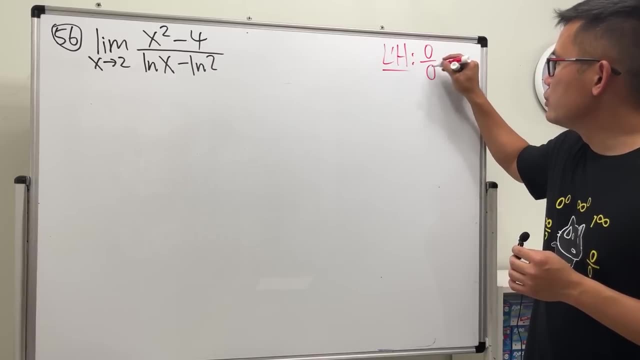 you guys, the so-called L'Hopital's rule. Keep in mind, the L'Hopital's rule says so. I just abbreviate it L'Hopital's rule. This right here: it's only good when we have 0 over 0. 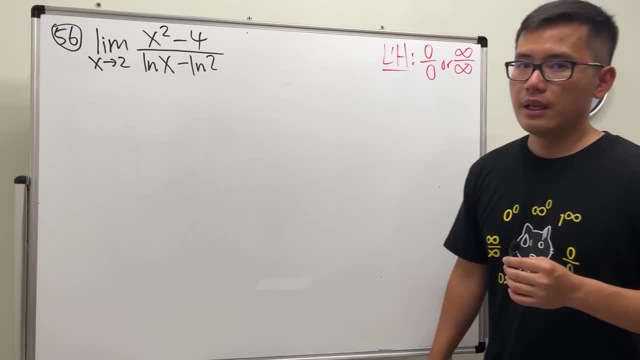 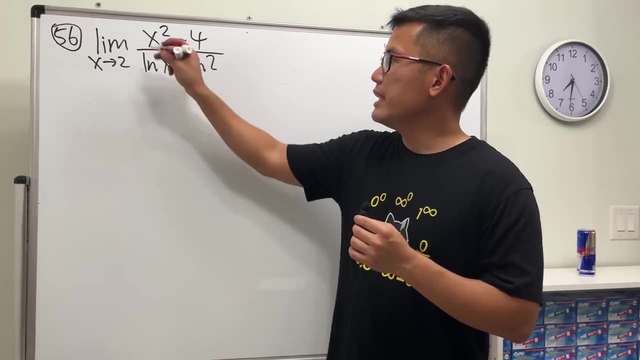 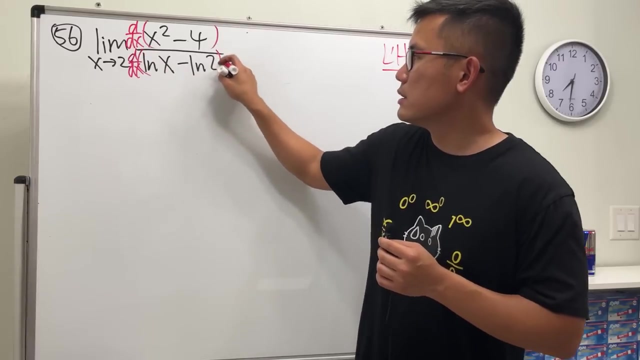 or infinity over infinity, And all you have to do is the following: Check: first We do have 0 over 0, so we get to use L'Hopital's rule, And then you just go ahead and do the derivative on the top, and then you do the derivative on the bottom, And that's the process. 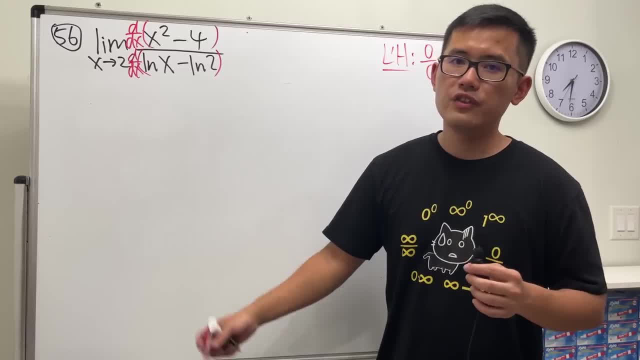 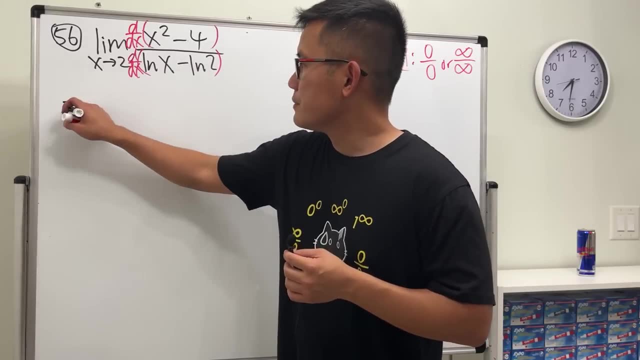 Okay, If it works, you have the answer, Everybody happy. If it doesn't work, too bad, We just have to think about it. if we want to do it, Anyway, let's see. This is the limit as x approaching 2.. Let me just get the answer for you guys first, and I will explain why. 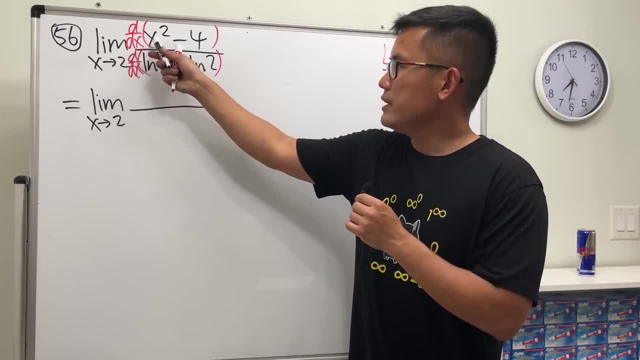 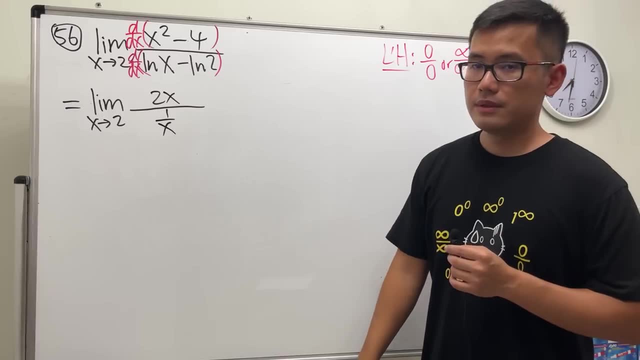 this is the case Differentiating x squared minus 4, we get 2x. And then take the derivative of ln x, we get 1 over x. Okay, So again it's just the derivative of the top, Yeah, And then you do the derivative of the bottom, And then we have the derivative of. 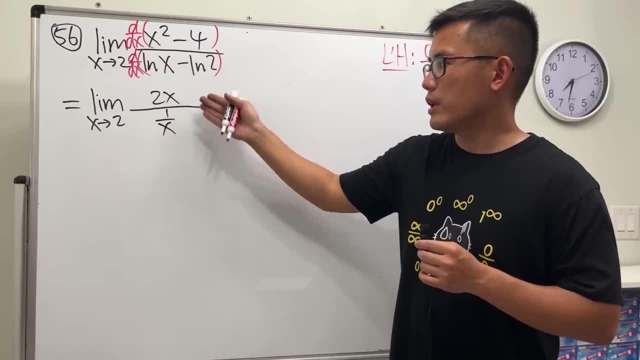 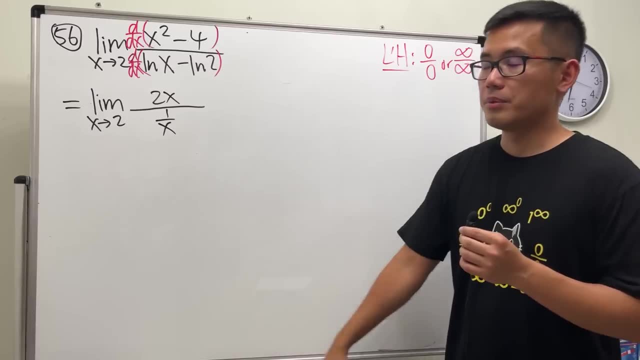 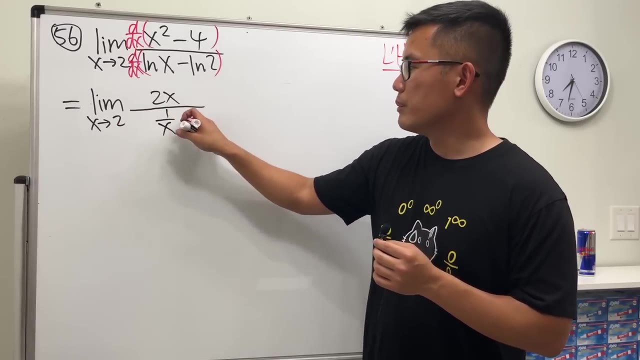 ln x, we get 1 over x. This is the number. that's why it's 0, so just that, right. So seriously, you will have to know your derivative really well in order to use L'Hopital's rule. Okay, Now we can put the 2 into the x's if you would like, or you would multiply. 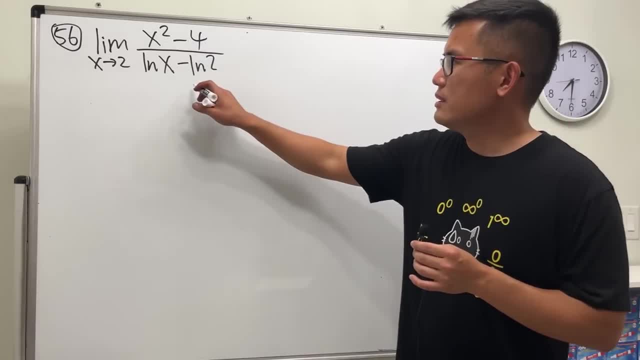 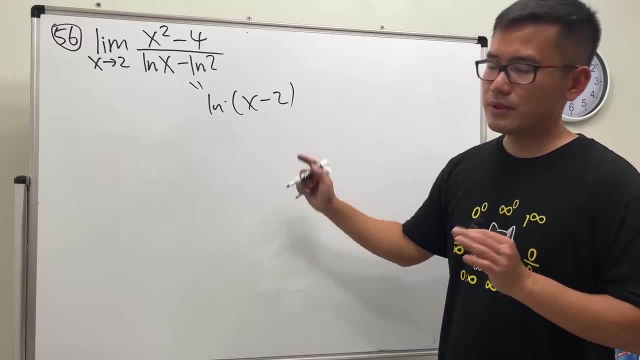 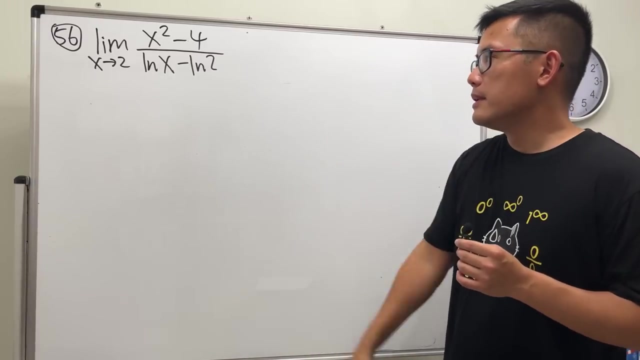 ln x minus ln 2. Is this just the same as ln and then x minus 2? No, No, Don't do that. It's not ln time. This is not even funny. No, Don't do that, No, No. 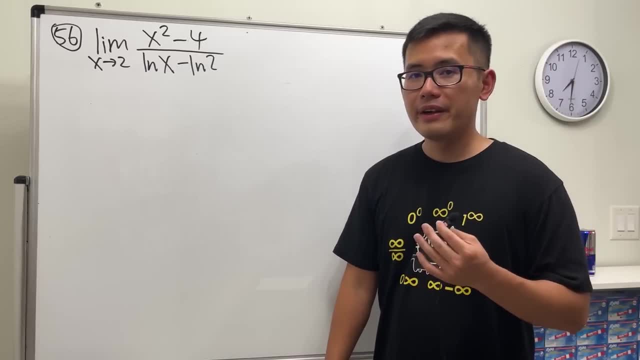 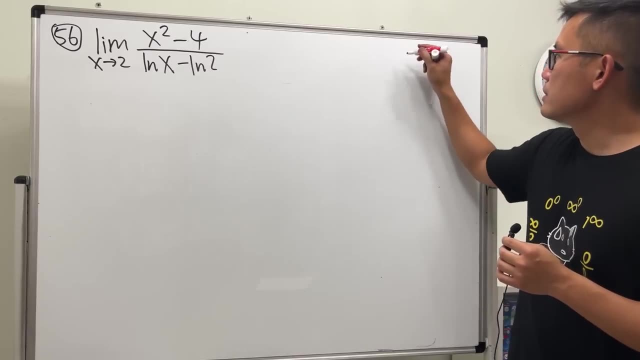 No. So here is the time that I'll show you guys the so called L'Hospital's Rule. Keep in mind, the L'Hospital's Rule says, so I'll just abbreviate it L'Hospital's Rule. This right here is only good when we have 0 over 0. 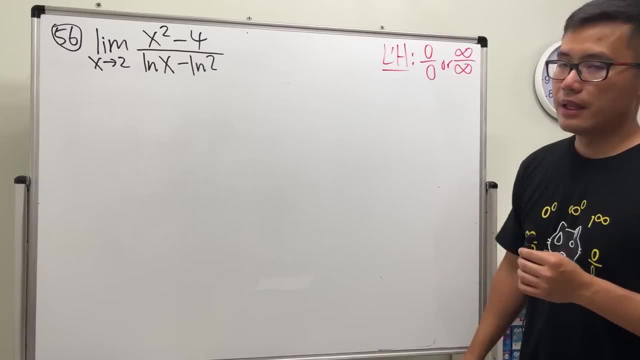 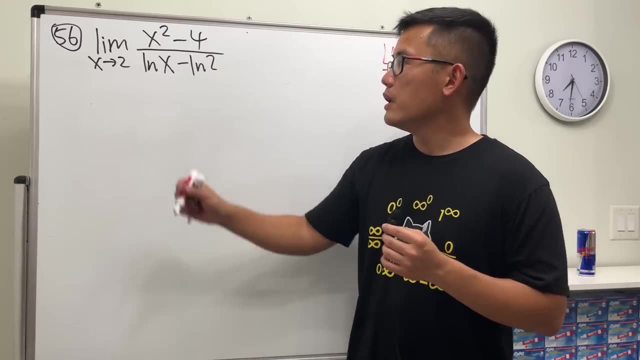 or infinity over infinity, and all you have to do is the following: check first we do have 0 over 0, so we get to use L'Hospital's Rule, and then you just go ahead and do this. you do the derivative on the top and then you do the derivative. 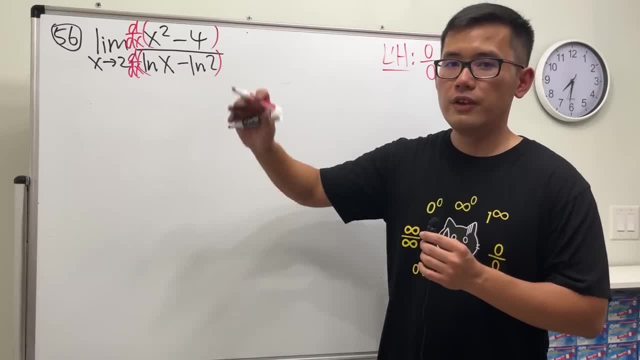 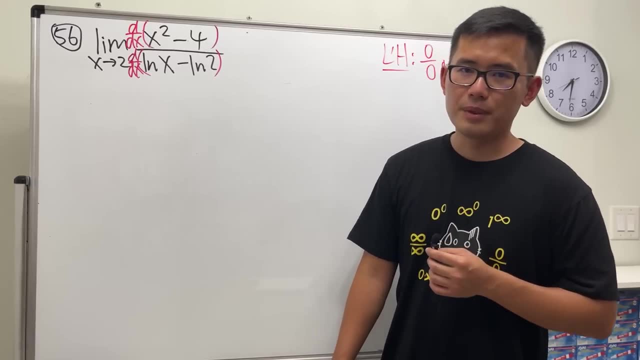 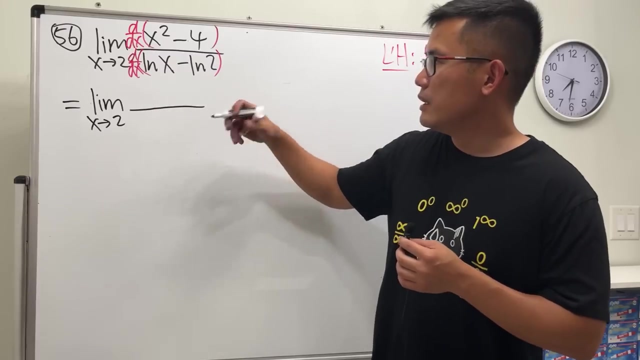 on the bottom and that's the process. if it works, you have the answer, everybody happy. if it doesn't work, too bad, we just have to think about it anyway. let's see, this is the limit. as x approaching 2, let me just get the answer for you guys first, 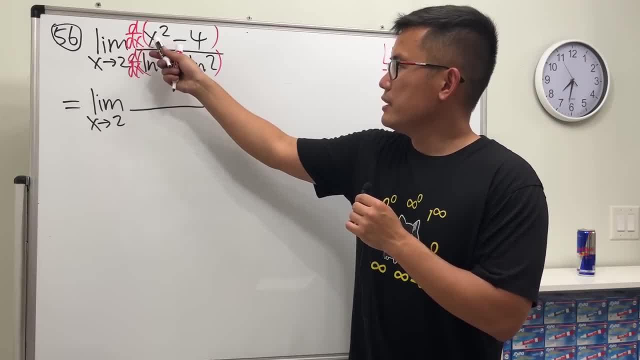 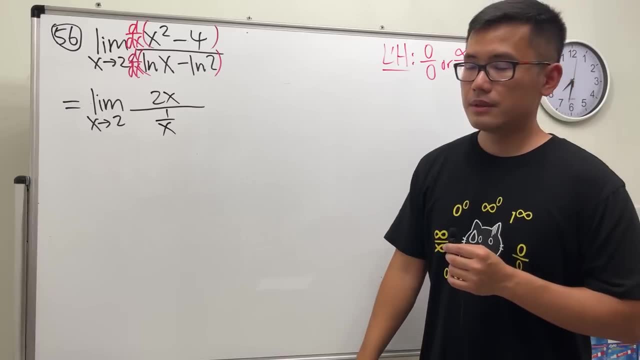 and I'll explain why this is the case. differentiating x squared minus 4, we get to x. and then take the derivative of ln x, we get 1 over x. so again, it's just the derivative of the top, and then you do the derivative of the bottom. 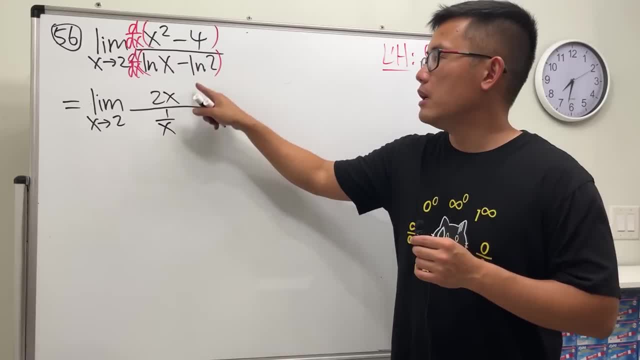 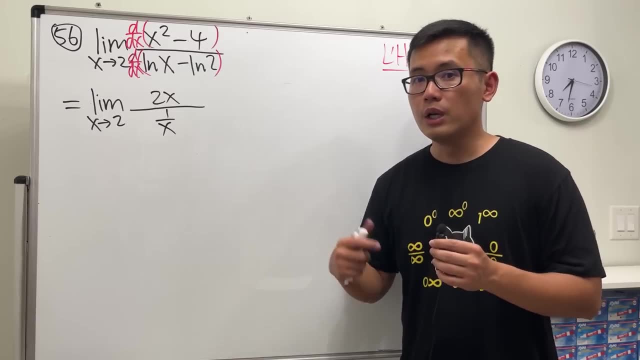 and the derivative of ln x is 1 over x. this is the number. that's why it's 0, so it's just that. so, seriously, you will have to know your derivative really well in order to use L'Hospital's Rule. ok, now we can put the 2. 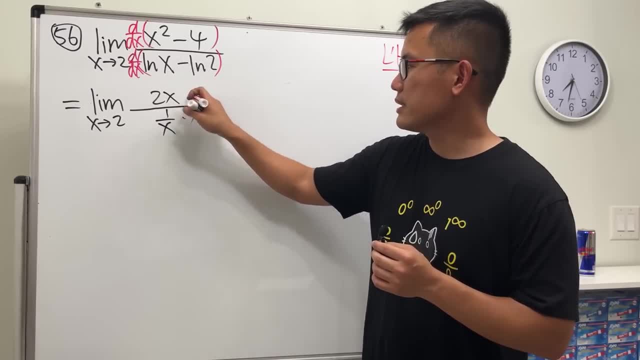 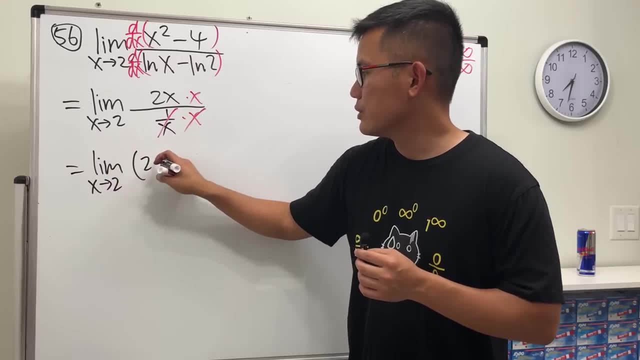 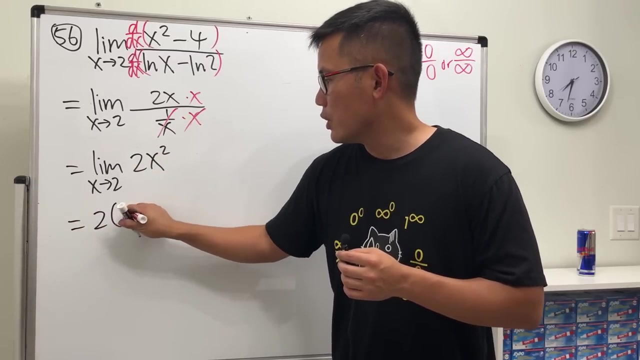 into the x's if you would like. or you can multiply x and x. just simplify first. so this is the same as limit x approaching 2 and just 2x squared. yeah, and then just work it out. so it's 2 times 2 squared. 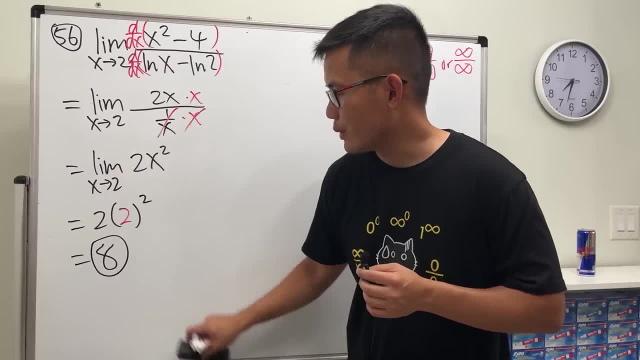 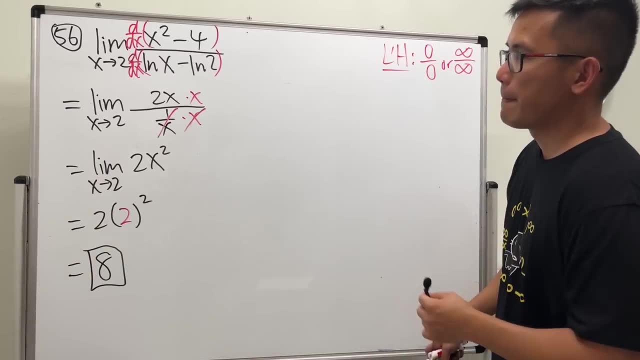 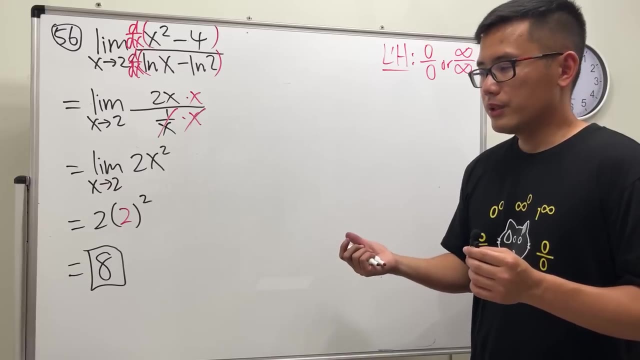 4 times 2, which is 8. yeah, why do you have to circle it? I usually box it, sorry. alright, cool, done now. here is the reason why this works. first, I want to tell you guys that a lot of mathematicians they do not like. 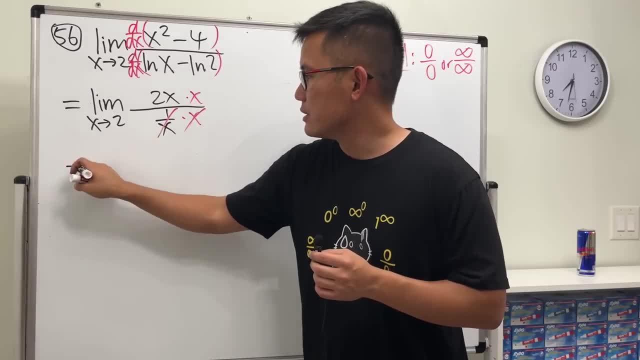 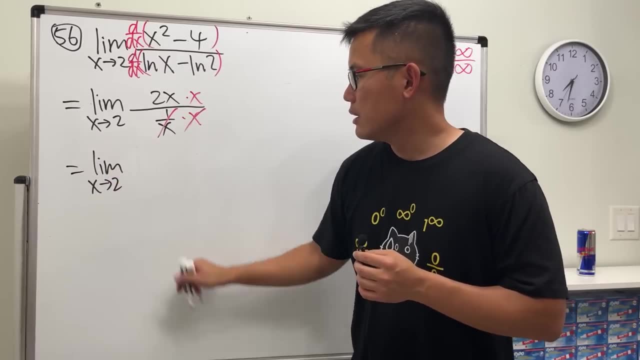 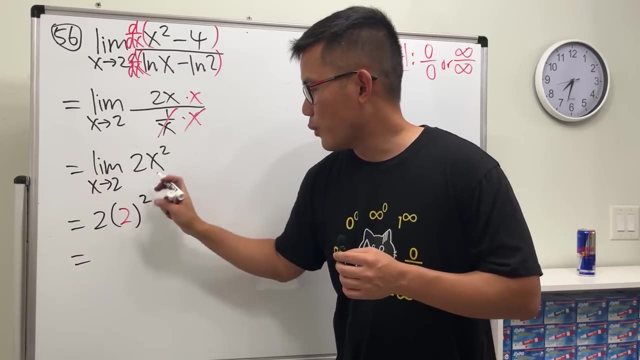 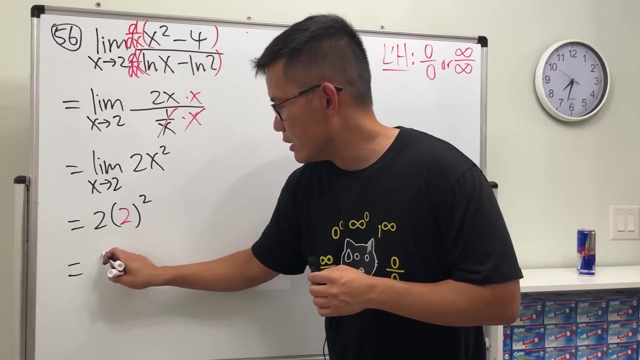 the x and and x. just simplify it first. So this is the same as the limit, x approaching 2.. just 2x squared, yeah, and then just worked out right. so it's two times two squared four times two, which is eight. yeah, why do you circle it? i usually box it. sorry. all right, cool done. 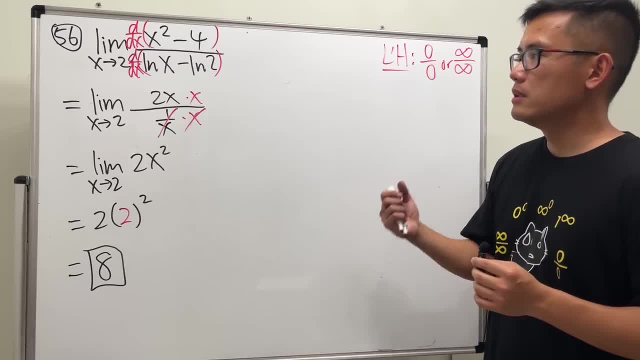 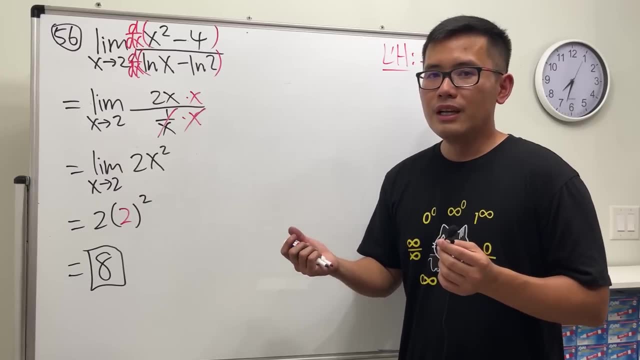 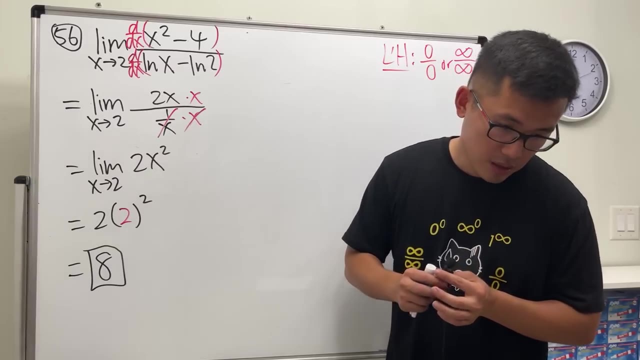 now here is the reason why this works. first i want to tell you guys that a lot of mathematicians they do not like the l'hopital's rule. sometimes i hate it too because it caused the circular reasoning. i'll explain that in the next category. 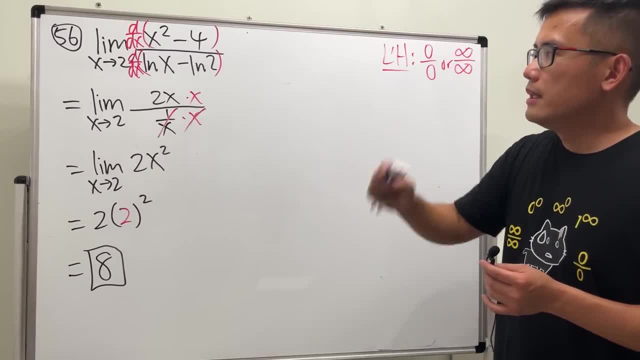 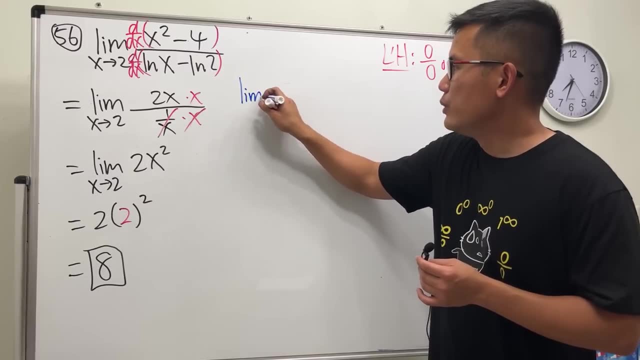 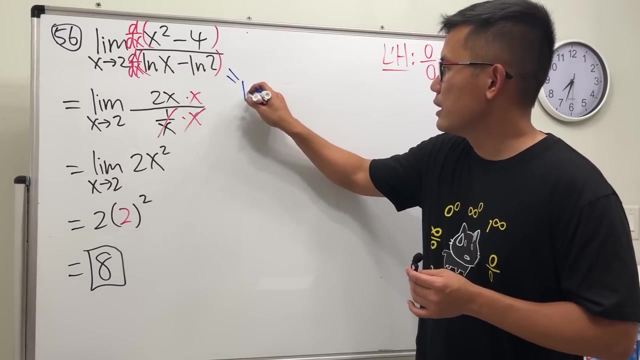 but let's, let's see to explain why this works. it's just that you will have to do this the long way and then i'll just tell you if we look at the limit. let me just rewrite this again. so let me just rewrite this right here. right, if we have the 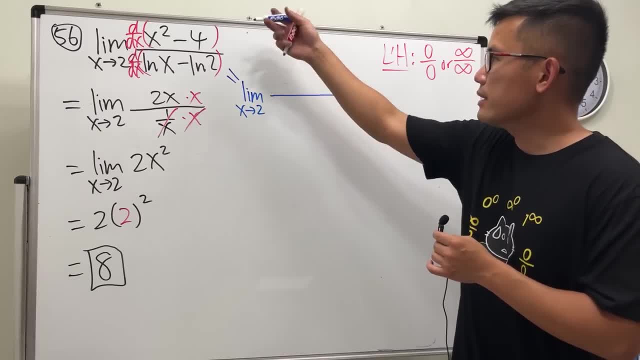 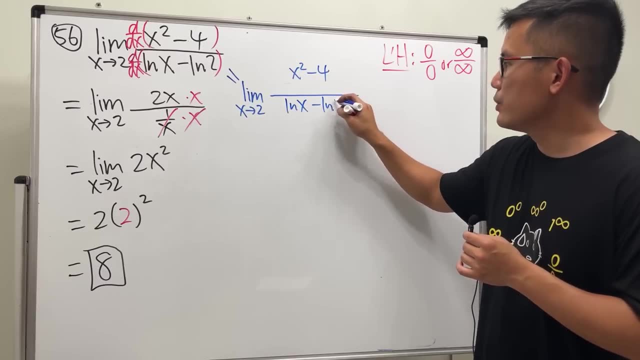 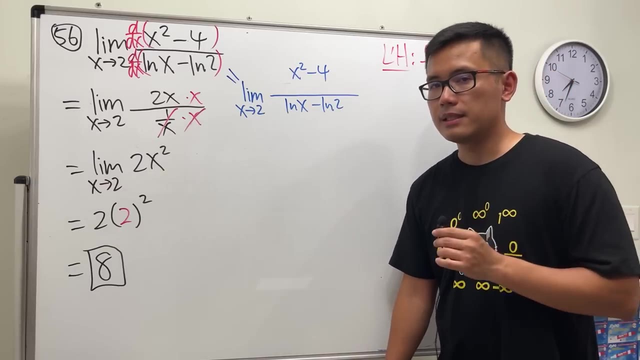 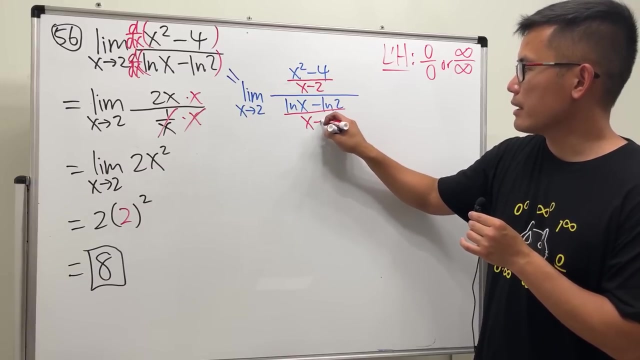 limit as x approaching two. and then on the top we have x squared minus four, yeah, and on the bottom we have ln x minus ln two. right looks good? not really, because it's zero for zero. but let's do the following: i'm going to divide the top by x minus two. likewise, we'll do the same on the bottom. 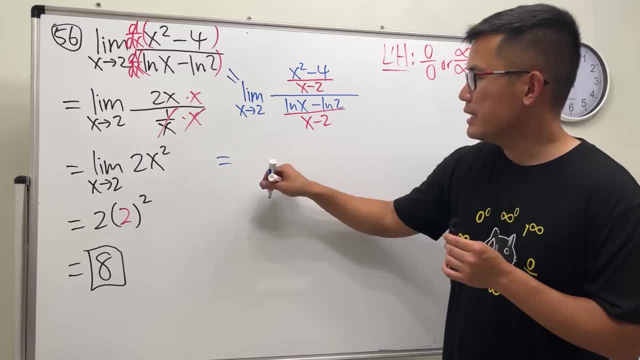 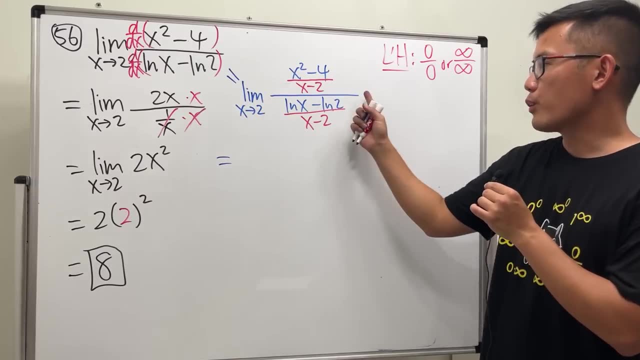 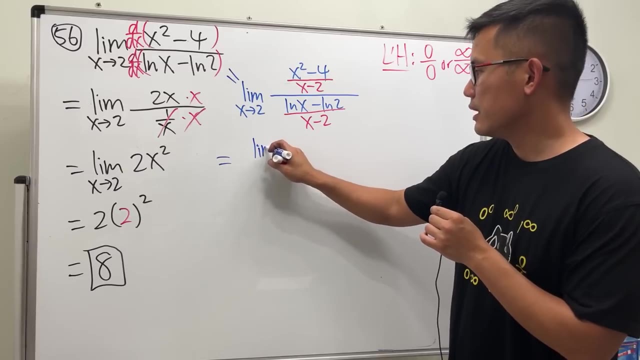 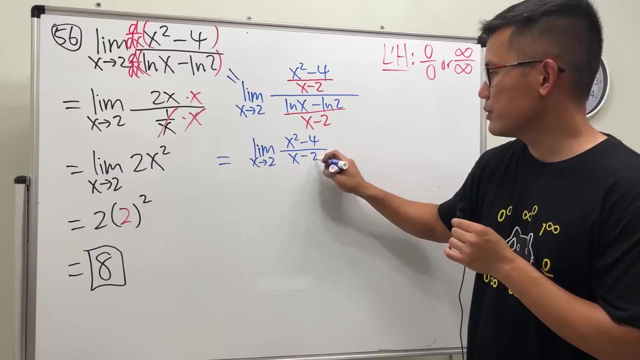 as well. and then i'm going to read this as: do the limit on the top and then divide the limit on the bottom. and we can do so because the limit of a quotient is a quotient of the limit, assuming they both exist. so this is the same as saying the limit as x approaching two, x squared minus four over, x minus two and over. 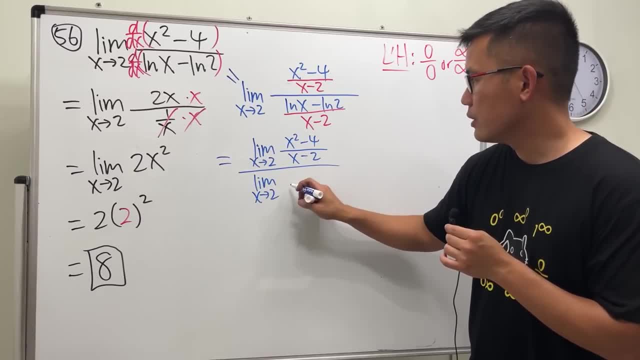 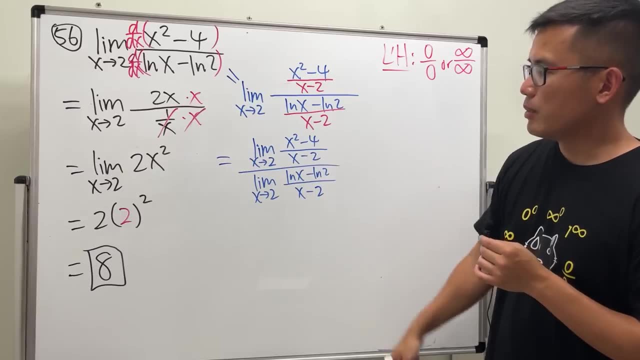 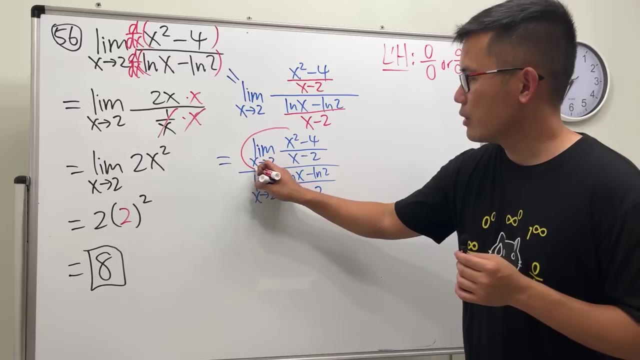 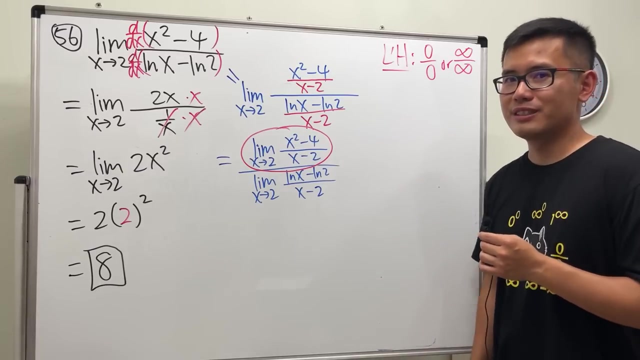 limit x approaching two, and then that. so again, the limit of a quotient is a quotient of a limit. provided they both exist, they do so. that's why we can do this. now, if you look at the top right here, what does this represent? i know we can solve this by using the algebraic limits, but if you 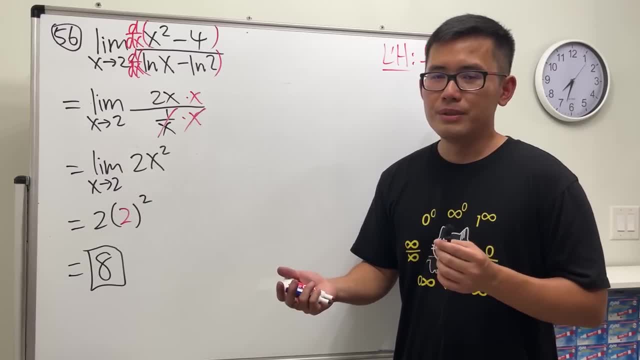 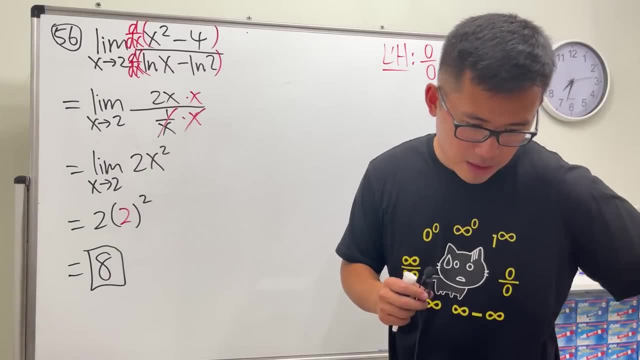 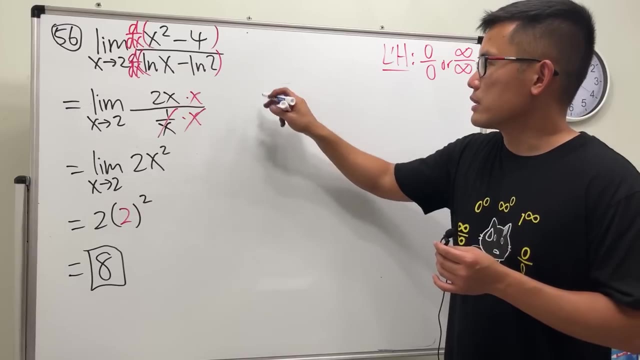 the L'Hospital's Rule. sometimes I hate it too because it cause the circular reasoning, and I will explain that in the next category. but let's see to explain why this works. it's just that you will have to do this the wrong way, and then I will just tell you. 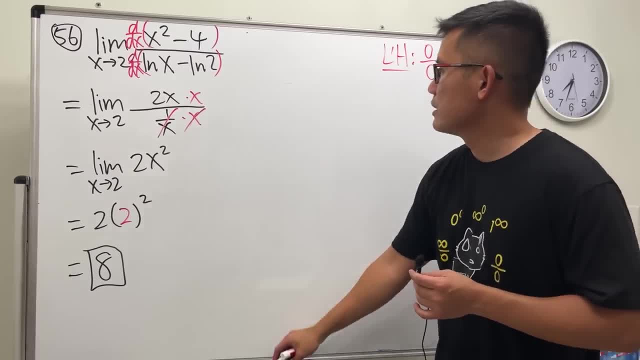 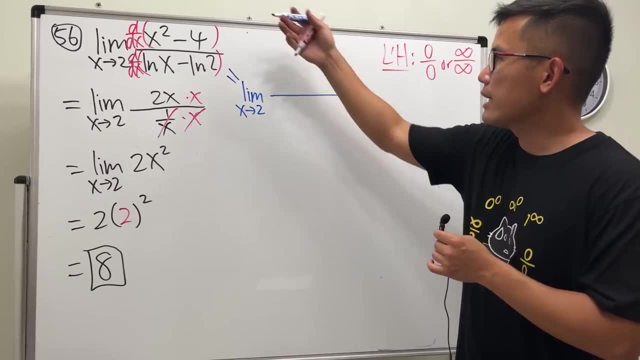 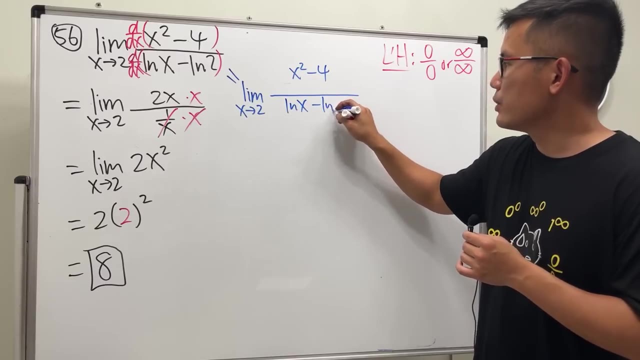 if we look at the limit- let me just rewrite this again. so let me just rewrite this right here- if we have the limit as x approaching 2, and then on the top we have x squared minus 4 and on the bottom we have ln x minus ln 2, 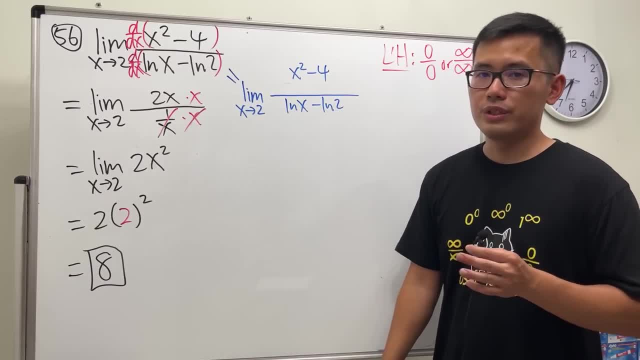 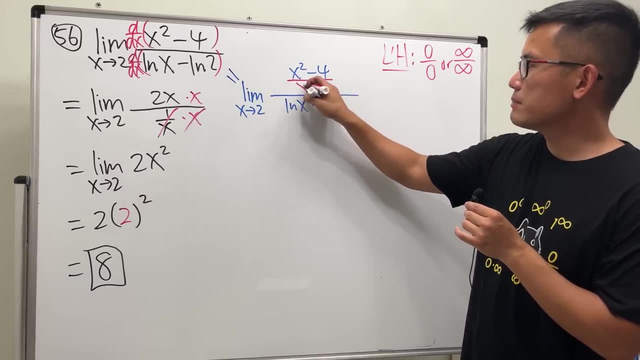 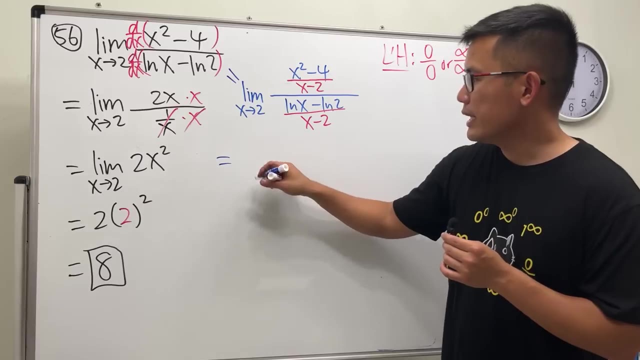 right looks good. not really, because it's 0 for 0, but let's do the following: I'm going to divide the top by x minus 2. likewise, we will do the same on the bottom as well, and then I'm going to read this as: 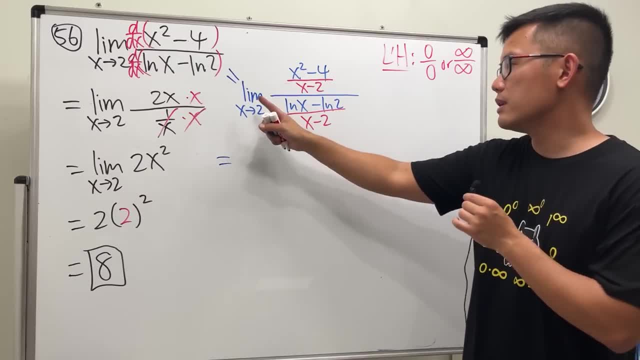 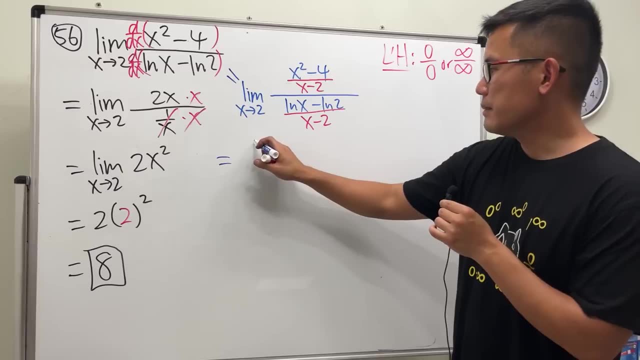 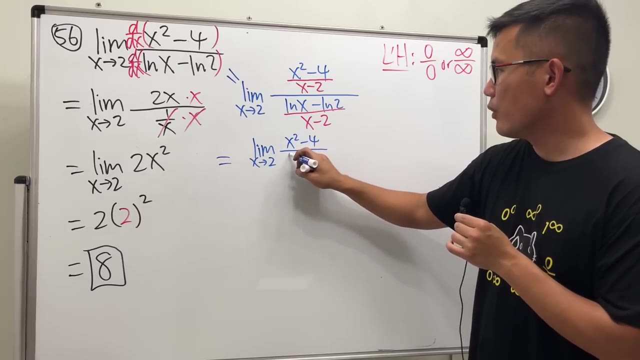 do the limit on the top and then divide the limit on the bottom. and we can do so because the limit of a quotient is a quotient of the limit, assuming they both exist. so this is the same as saying the limit as x approaching 2, x squared minus 4. 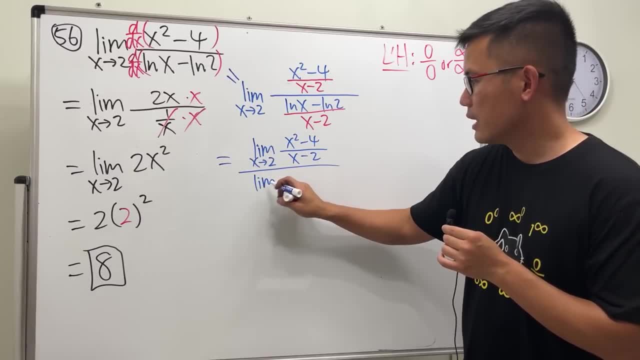 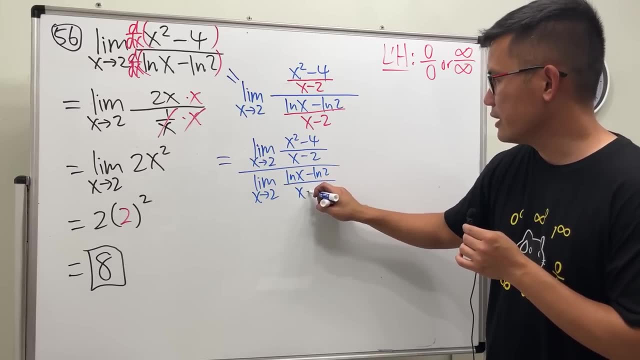 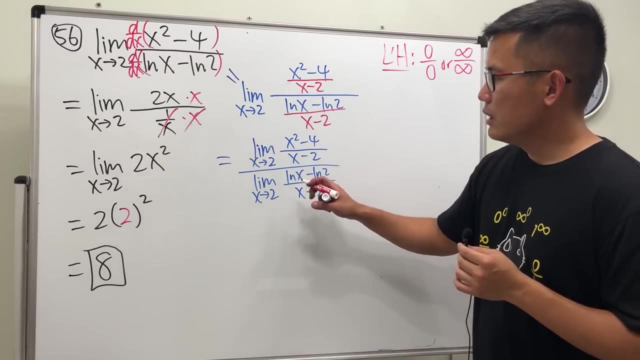 over x minus 2 and over limit x approaching 2. so again, the limit of a quotient is a quotient of a limit, provided they both exist. so that's why we can do this now. if you look at the top right here, what does this represent? I know we can solve this. 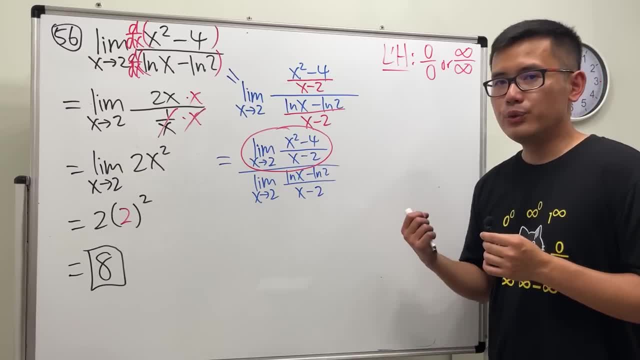 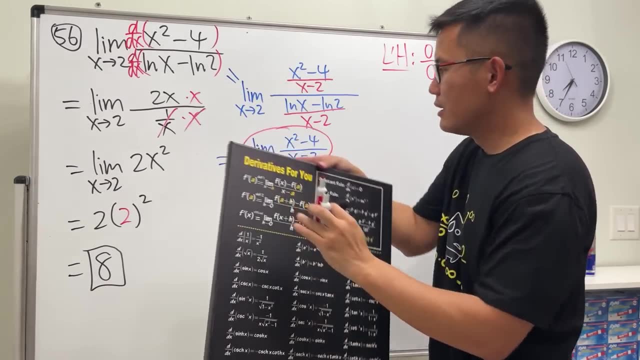 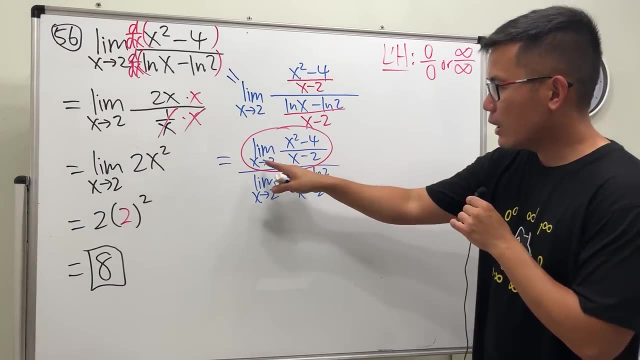 by using the algebraic limits. but if you remember the definition of derivative, and you know it, I'm going to bring this up right here. this thing, doesn't this remind you of a derivative? it does, huh, yes, and I would like to tell you, you see how we have: x is approaching 2. 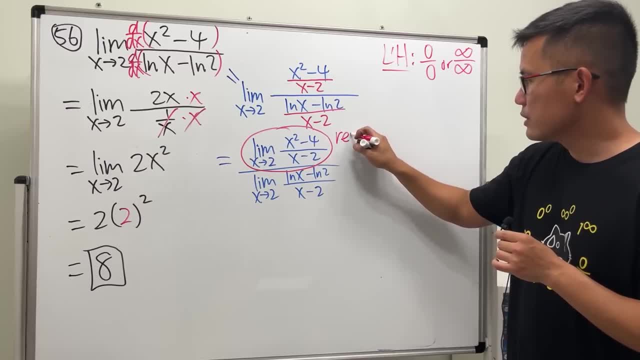 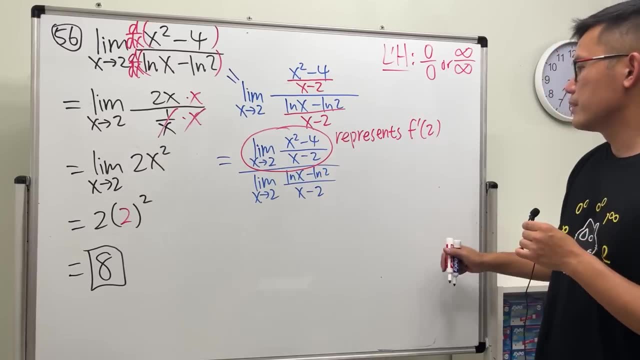 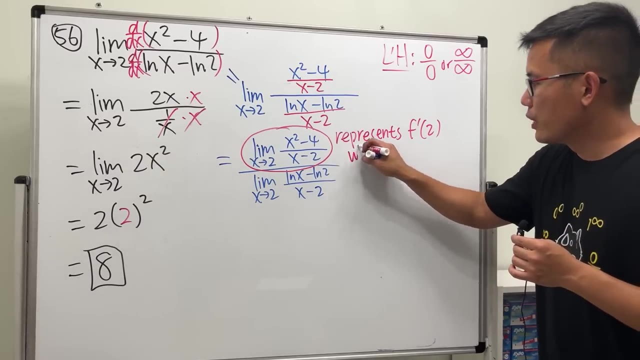 so I will tell you this right here: represents- I'll just spell it out for you guys: represents f prime of 2, because x is approaching 2, so it's a derivative of some function when x is 2. but what's the function, though, where the function 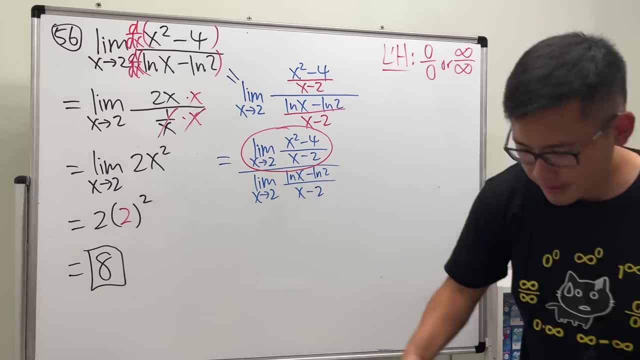 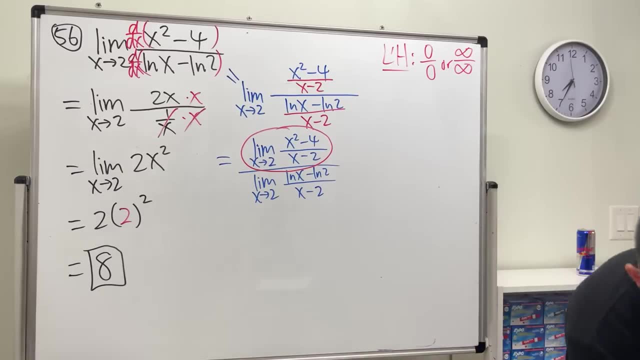 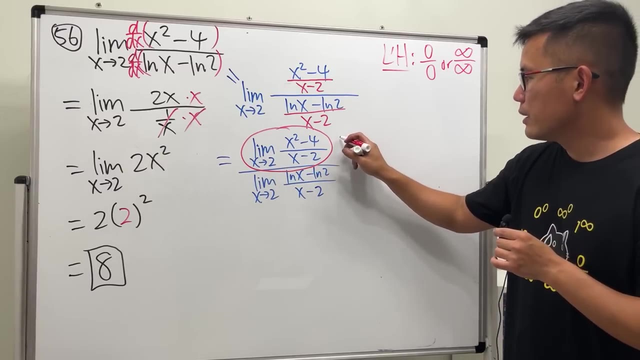 remember the definition of derivative, and you know it. i'm going to bring this up right here. this thing, doesn't this remind you of a derivative? it does, huh, yes, and i would like to tell you. you see how we have. x is approaching 2, so i will tell you this right here: represents- i'll just 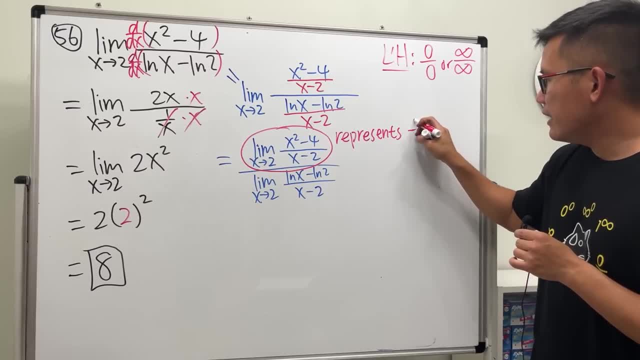 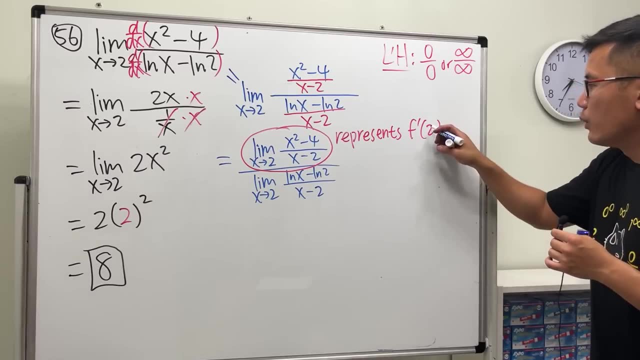 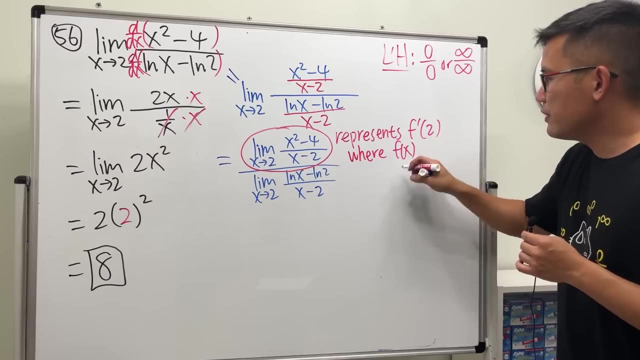 spell it out for you guys: represents f prime of 2, because x is approaching 2, so it's derivative of some function when x is 2. but what's the function, though? where the function? i'll just write it as f of x. it's just that. just x, square right, yes. 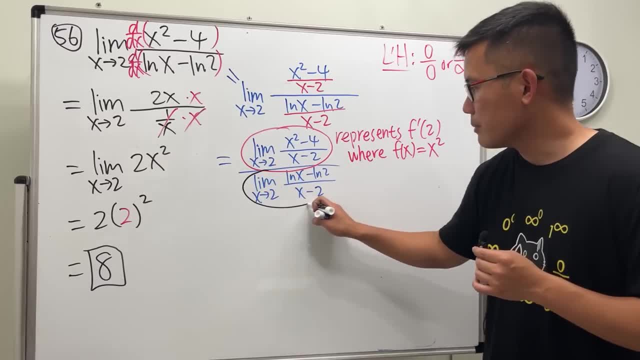 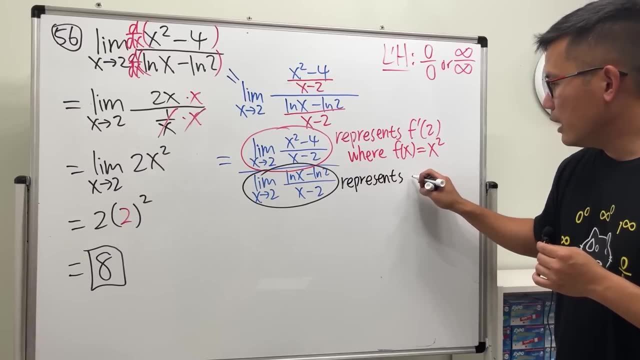 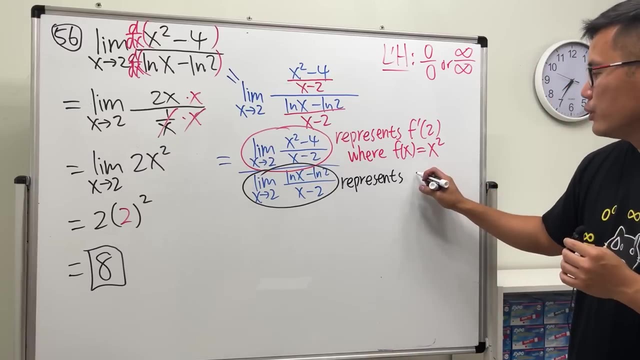 similarly we can also talk about the bottom right here. this right here represents again f prime of 2 as well, but i use f right here already, so just to reduce confusion, i'm going to use another letter, let's say g. just another function, right, because we're working on. 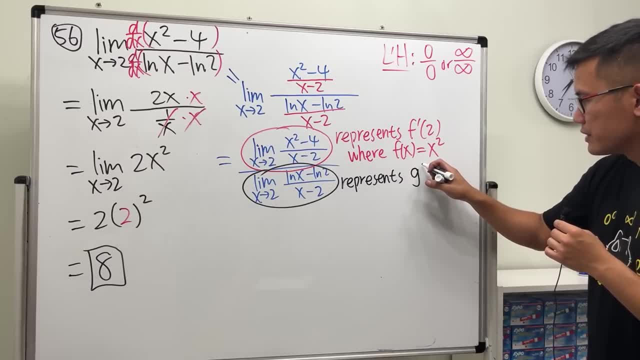 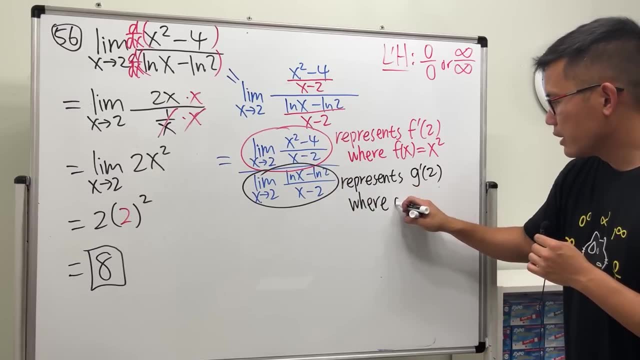 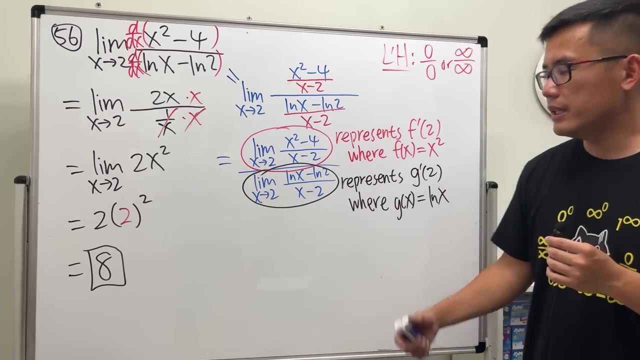 the same question. so let's use g: it's derivative of some function g. add 2, and then what the function is is just a function of some function g. and then what the function is is just a function just l and x. so where g of x equals l and x. so in fact the top is a derivative equation. likewise, 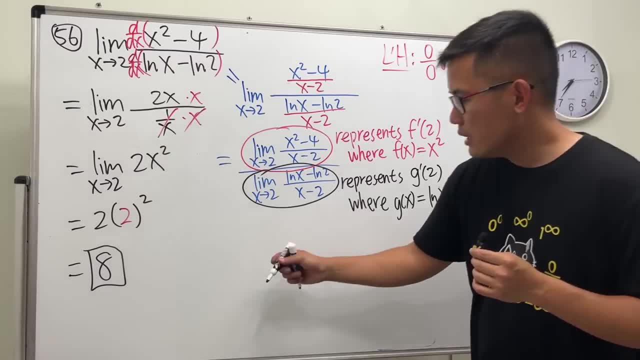 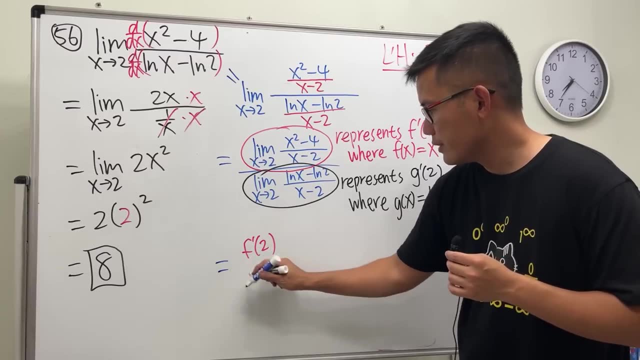 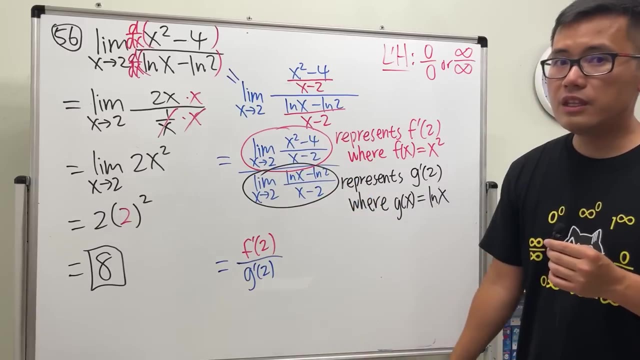 the bottom is also a derivative equation and you see, this right here is really just f prime of 2 over g prime of 2, so it's just a derivative of the top divided by the derivative of the bottom. assuming that the bottom is a derivative of the top. 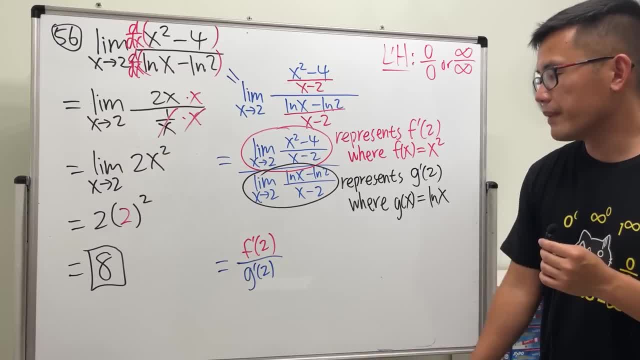 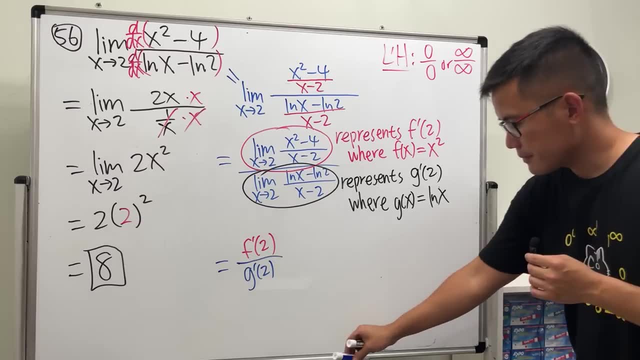 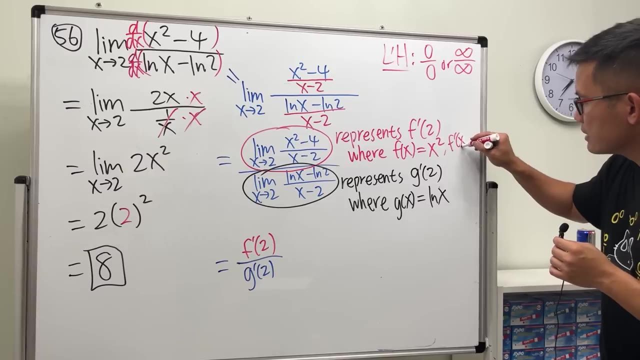 assuming that we get a nice answer for this. right, it does so, yeah. so what's f prime of 2, though? well, if you look at this carefully, you see that we know f of x is x squared, so this means f prime of x is just 2x, so this means f prime of 2. 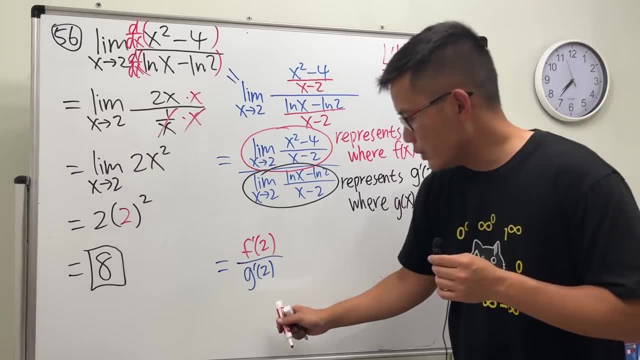 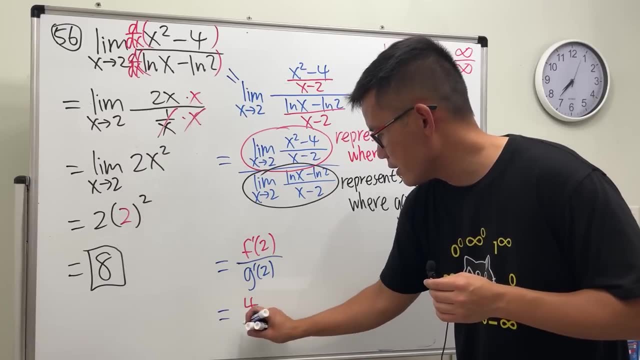 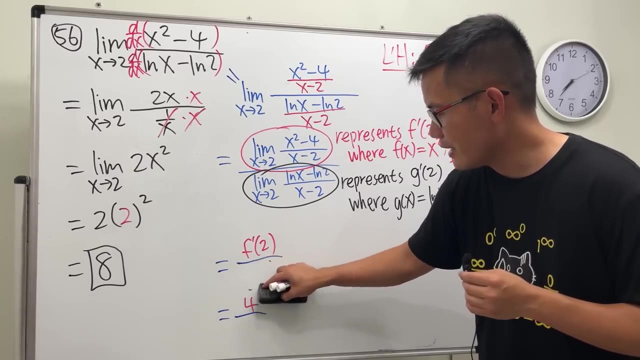 is just 2 times 2, which is 4.. so on the top here we actually just get a 4. on the top here we only get a 4, and on the bottom, as we saw earlier, this thing right here represents g prime of 2, and yes, I'm changing the color to make it prettier for you guys. 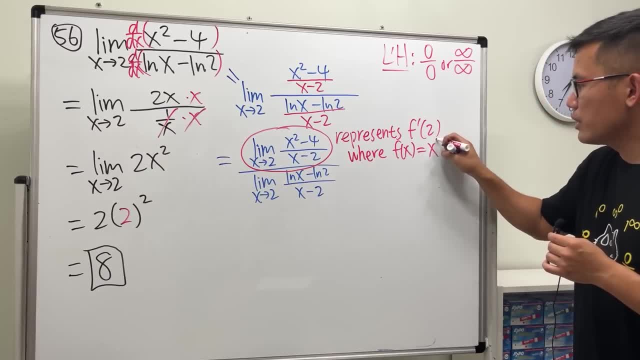 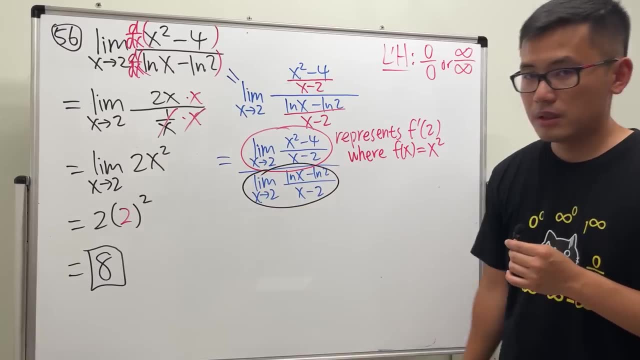 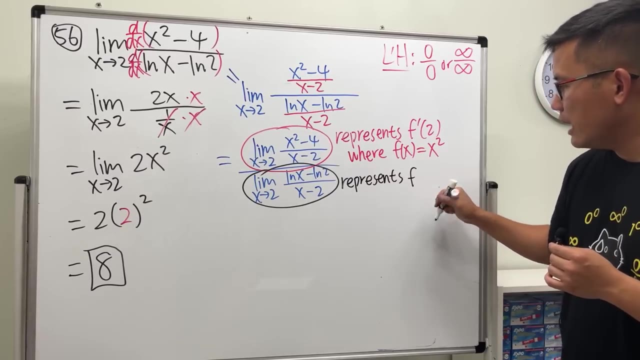 I'll just write it as f of x, which is x squared right. yes, similarly we can also talk about the bottom right here. this right here represents again f, prime of 2 as well, but I used f right here already, so just to reduce confusion I'm going to use another letter, let's say g. 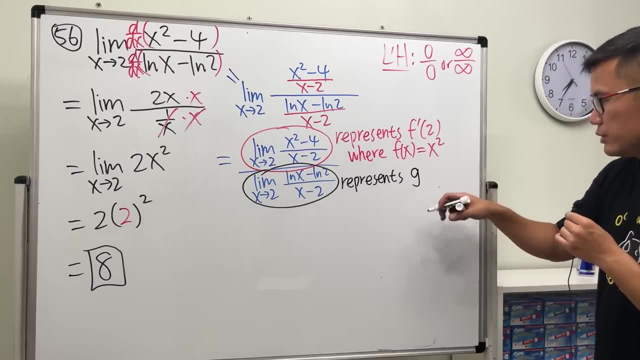 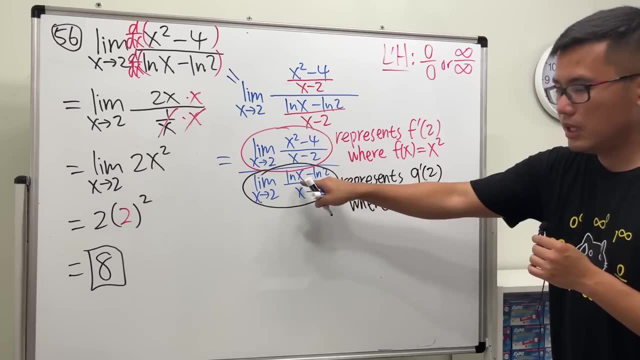 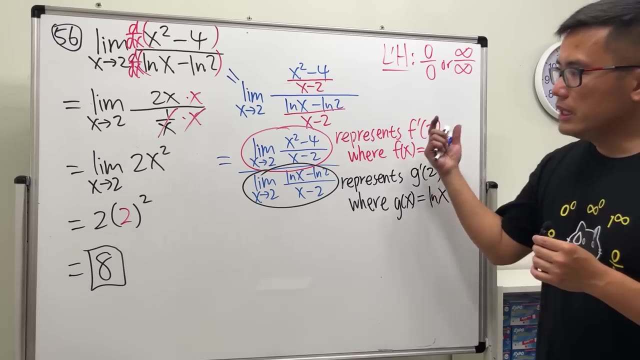 just another function, right, because we're working on the same question. so let's use g at 2 and then what the function is is just ln x, so where g of x equals ln x. so in fact the top is a derivative equation. likewise, the bottom is also a derivative equation. 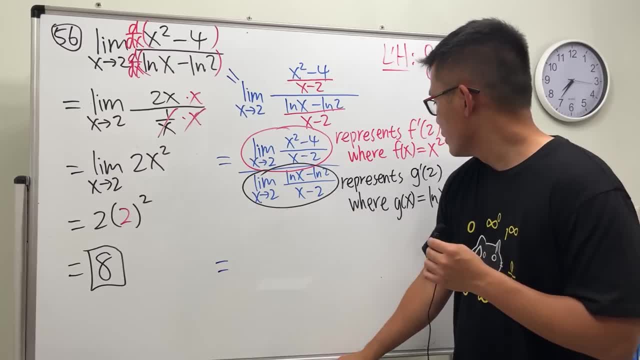 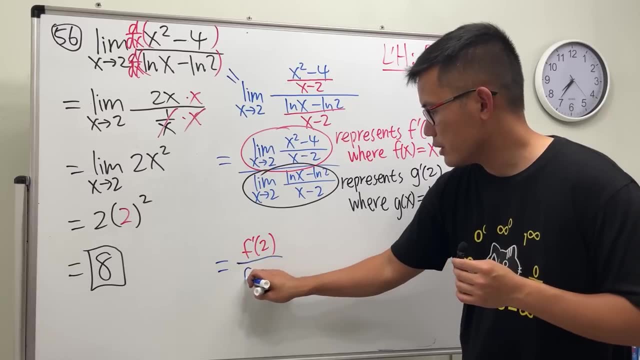 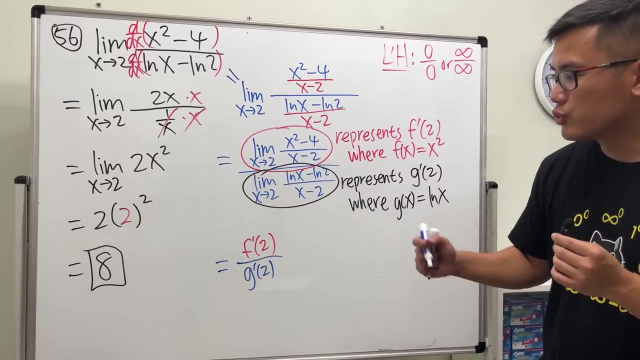 and you see this right here is really just f prime of 2 over g prime of 2, so it's just a derivative of the top divided by the derivative of the bottom. assuming that we get a nice answer for this, right, it does so, yeah. so what's f prime of 2, though? 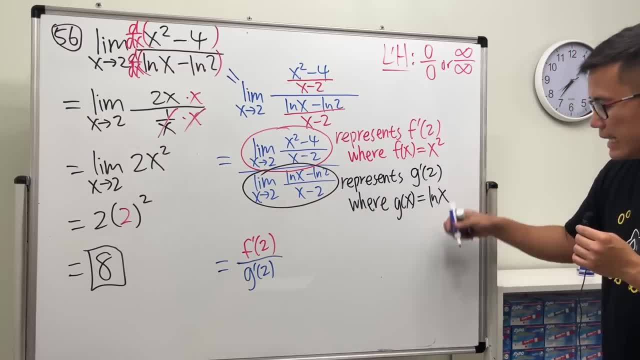 well, if you look at this carefully, you see that we know f of x is x squared. so this means f prime of x is just 2x. so this means f prime of 2 is just 2 times 2, which is 4. so on the top, here we actually just get. 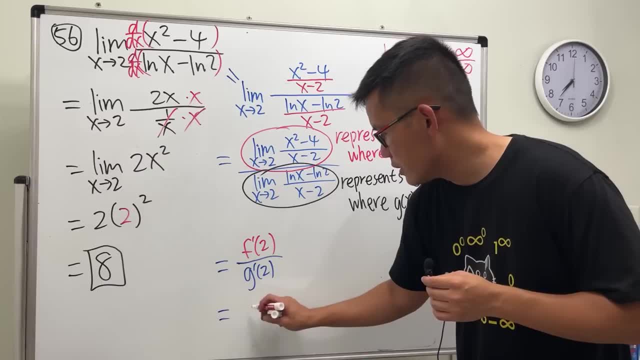 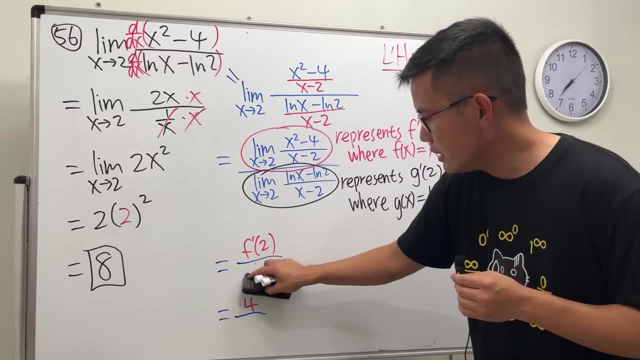 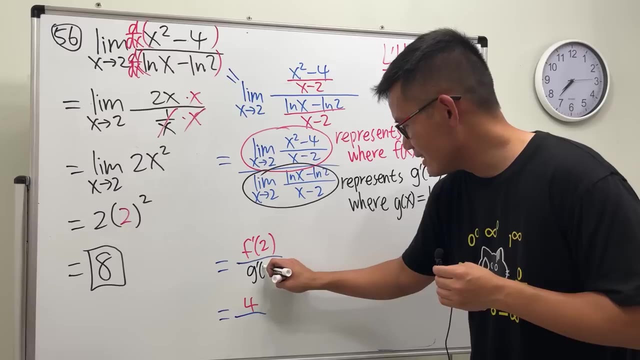 a 4. on the top here we just get a 4, and on the bottom, as we saw earlier, this thing right here represents g, prime of 2, and yes, i'm changing the color to make it prettier for you guys. and now you see, this is g of x is. 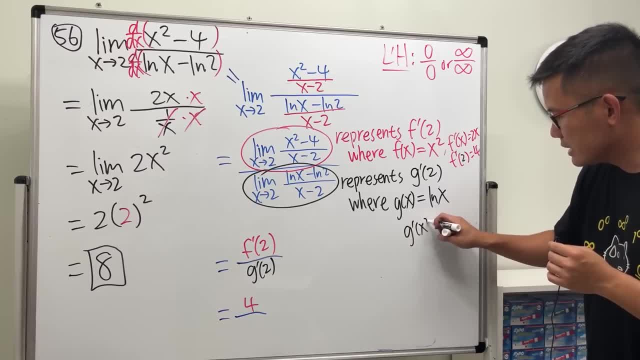 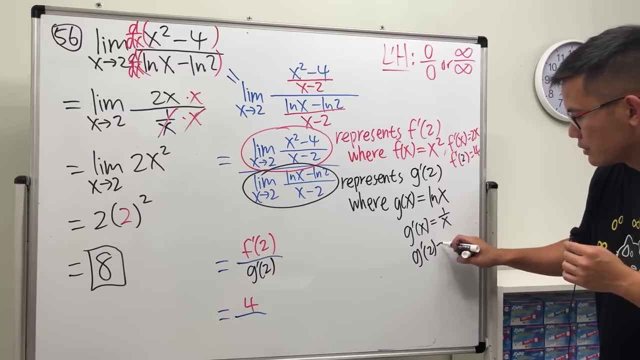 ln x. so we have to know our derivative g prime of x is just 1 over x. let's decipher with it right. and then we plug in 2, so it's just 1 over 2. so the bottom here is 1 half. simplify the fraction. 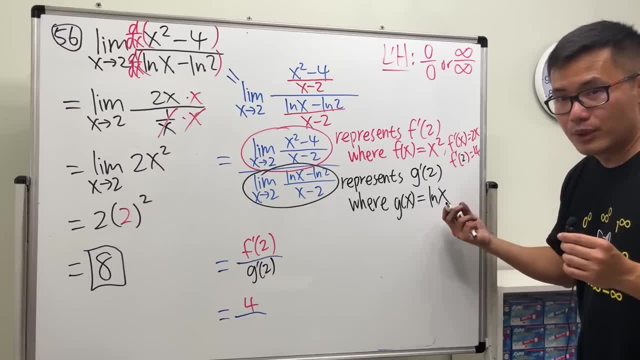 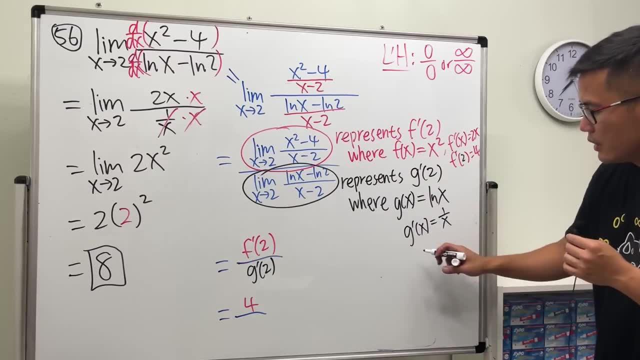 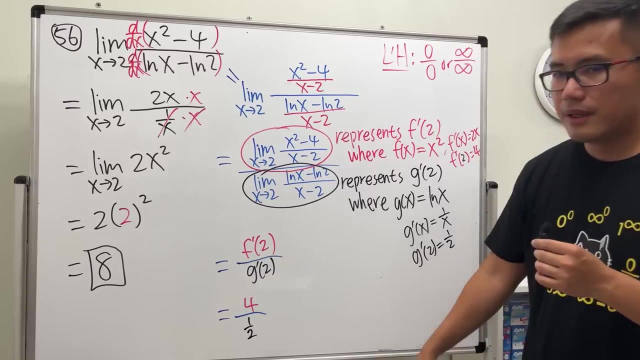 and now you see, this is g of x, is l and x. so we have to know our derivative g prime for x is just one over x. let's decide what we did right, and then we plug in two, so it's just one over two. so the bottom here is one half. simplify the fraction, multiply two and two. 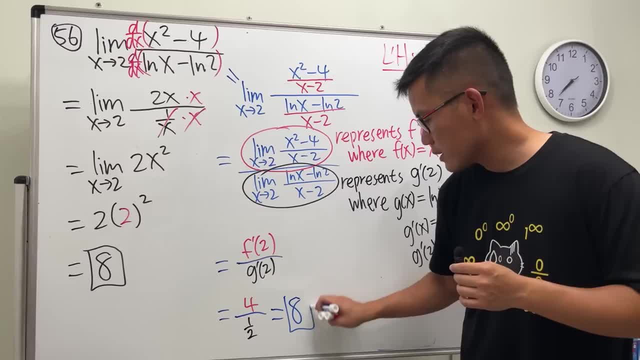 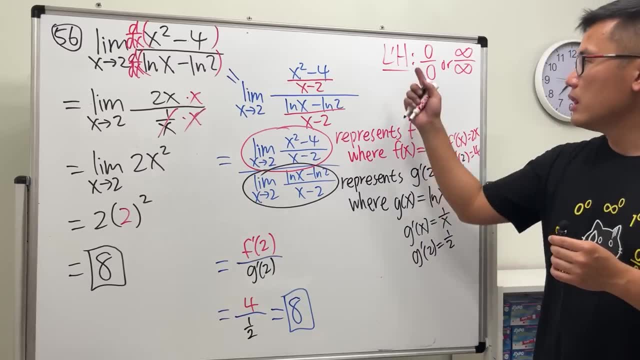 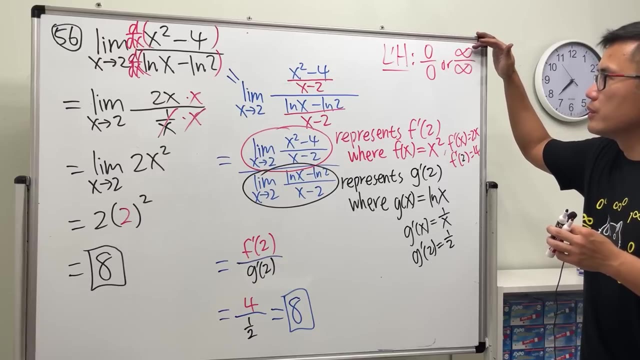 so, ladies and gentlemen, we end up with eight. yeah, so this is the idea behind the, the so-called lapito's rule, and again, we use. it's useful when we have zero over zero and also infinity. we can only use lapito's rule when we have zero for zero or infinity of infinity. however, 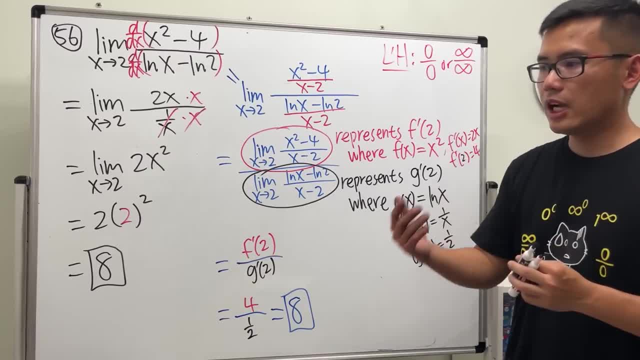 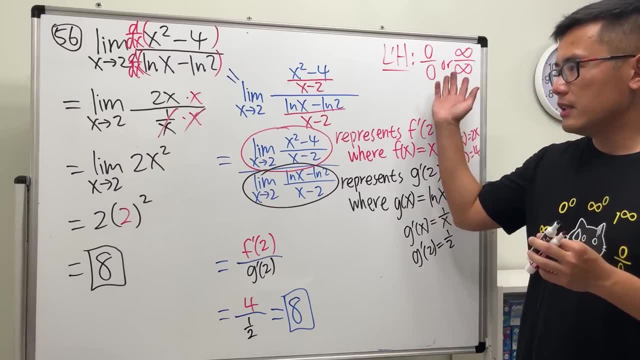 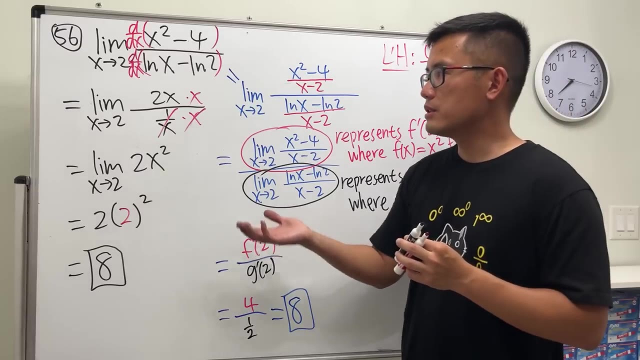 there might be some cases that lapito's rule does not help us get the answer. in that case you just have to try other things. but if you don't have this in the independent form, then cannot use lapito's rule and the reason why there are a lot of mathematicians don't like the lapido's rule. 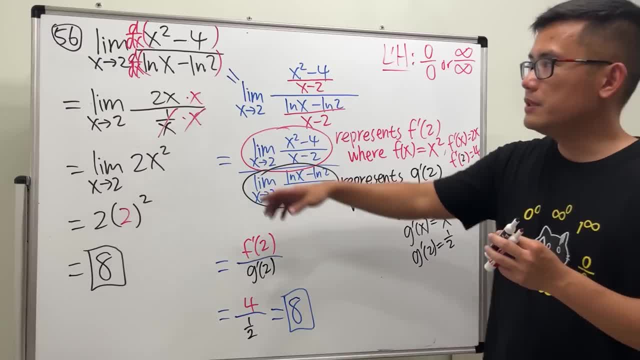 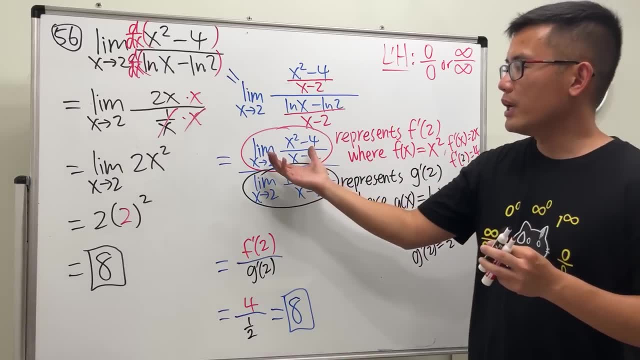 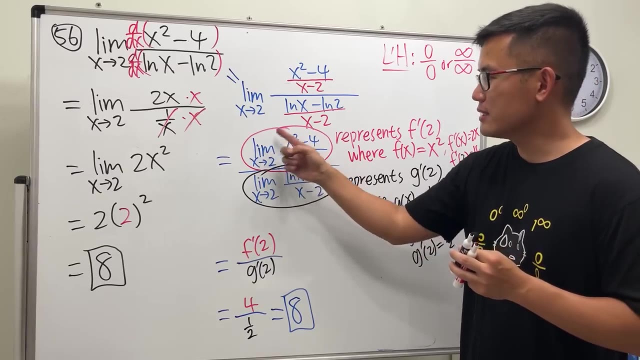 because he calls circular reasoning is because you see how, when we are doing limits we are using derivative, but when we are trying to get the derivative we will have to use limit. see earlier. when i show you guys this, i can actually tell you: hey, let's just do the derivative. no, we have to do it algebraically. 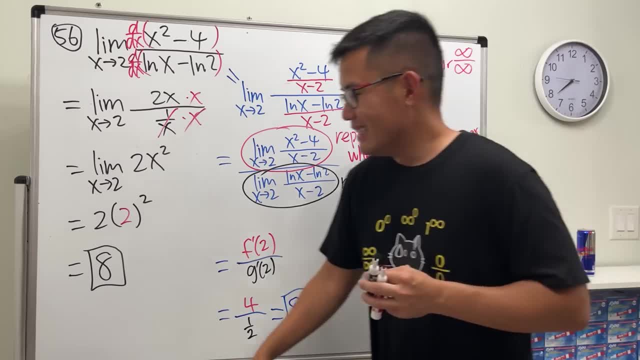 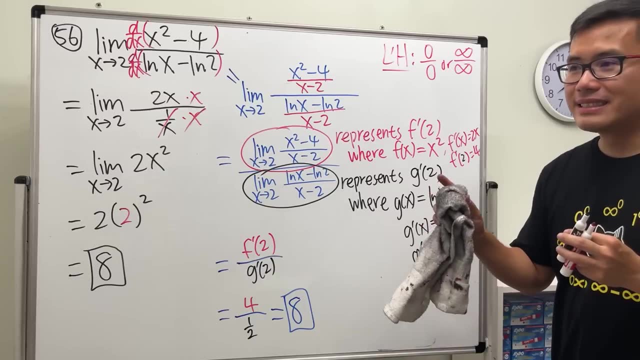 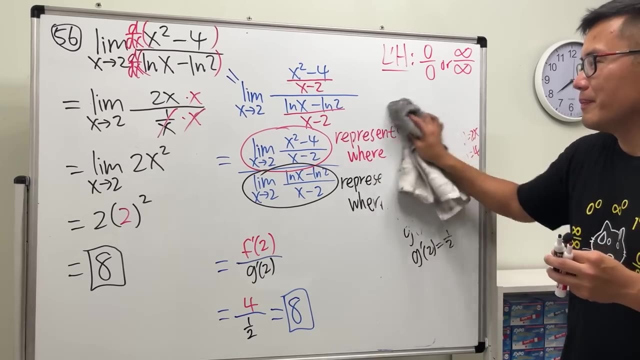 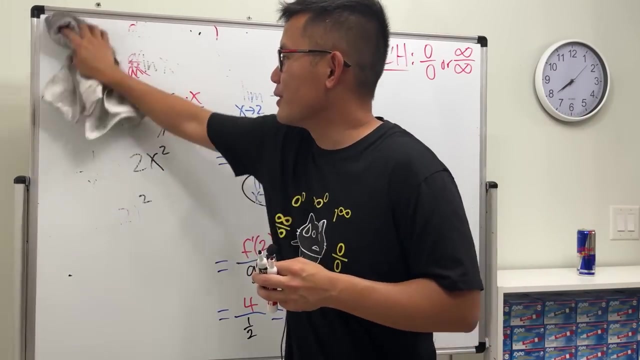 first, yeah, so yeah, be be really careful. i will tell you, though, the best time for us to use lapito's rule is infinity over infinity, but then still. a lot of people will still not like it too much, but it's convenient. i will say, yeah, that's an explanation, because i want to move on. 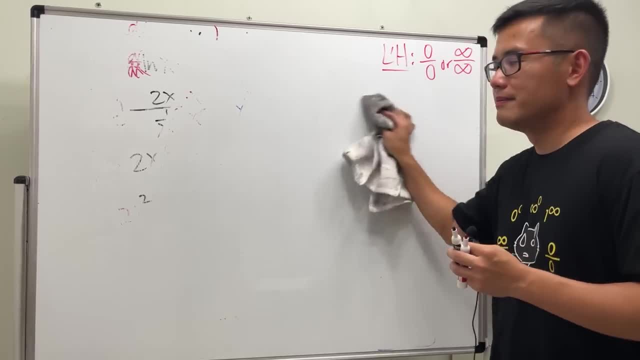 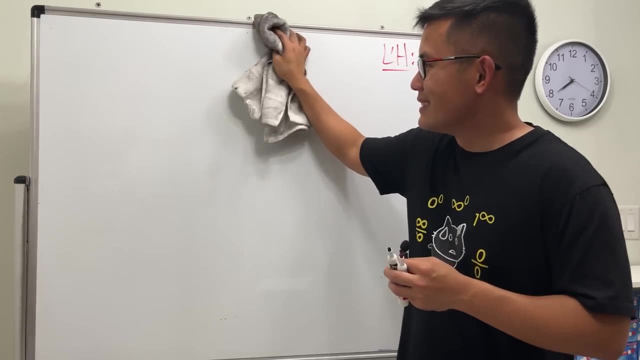 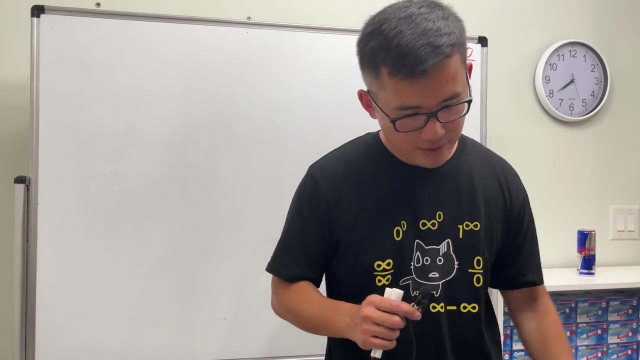 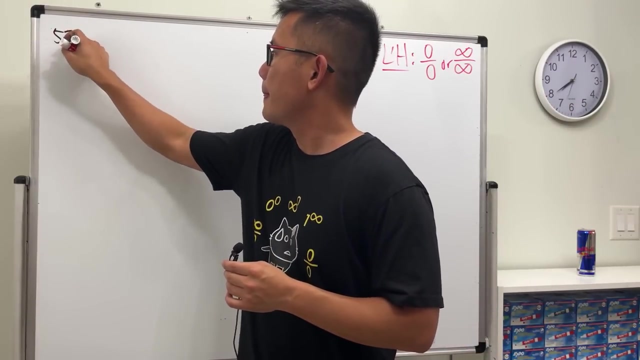 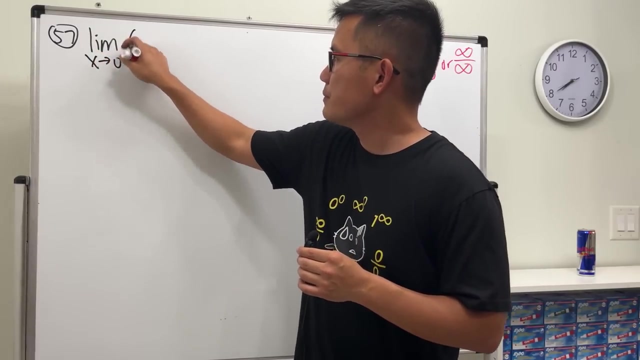 and usually i would say i want to go home, but i'm home already, so it's not like when i was doing that. 100 integral or 100 derivative questions: okay, number 56, no. number 57 limit. give you guys a tough one. x approaching zero, and then we have one over x. 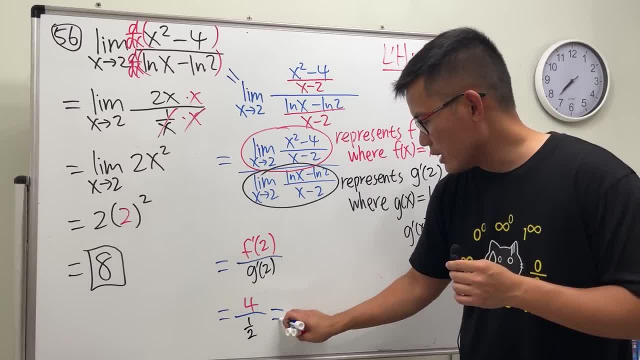 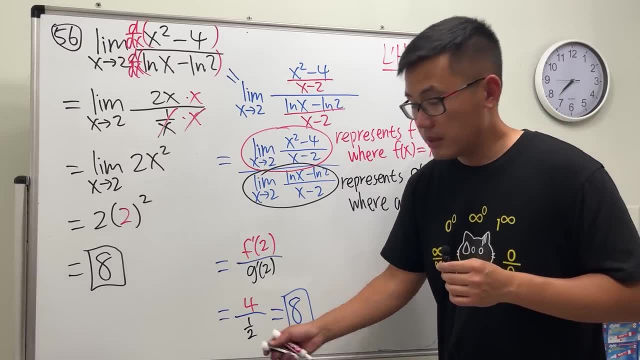 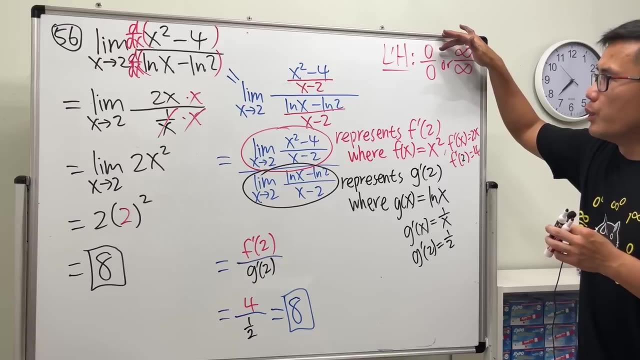 multiply 2 and 2, so, ladies and gentlemen, we end up with 8. yeah, so this is the idea behind the, the so called Lapito's rule, and again it use it's use for when we have 0 over 0 and also infinity. we can only use Lapito's rule when we have 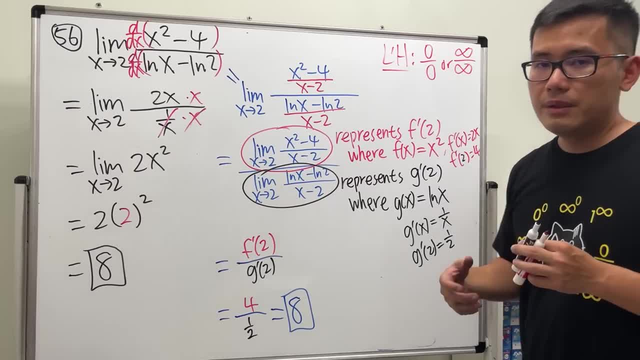 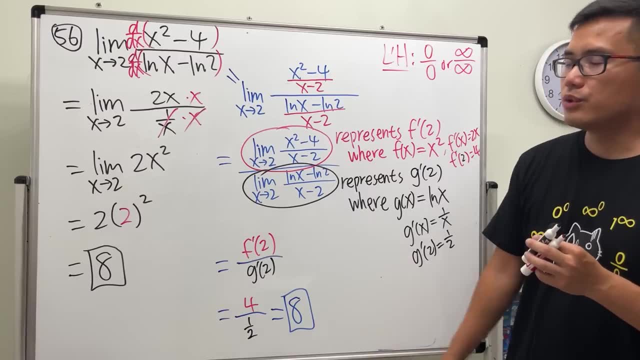 0 over 0 or infinity over infinity. however, there might be some cases that Lapito's rule does not help us get the answer. in that case, you just have to try other things. but if you don't have this independent form, then you cannot use Lapito's rule. 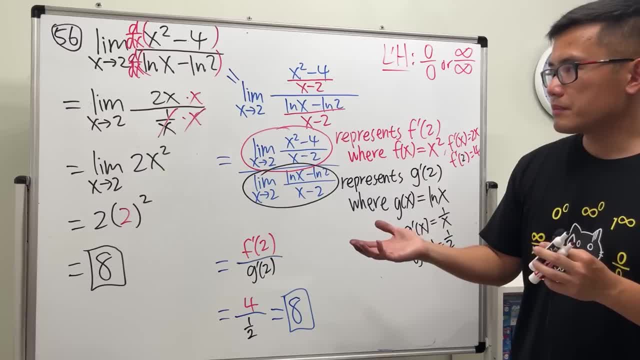 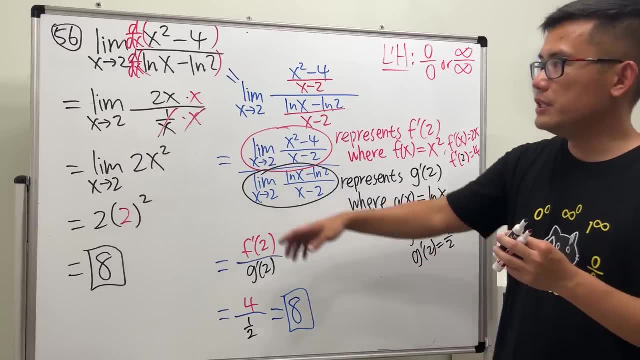 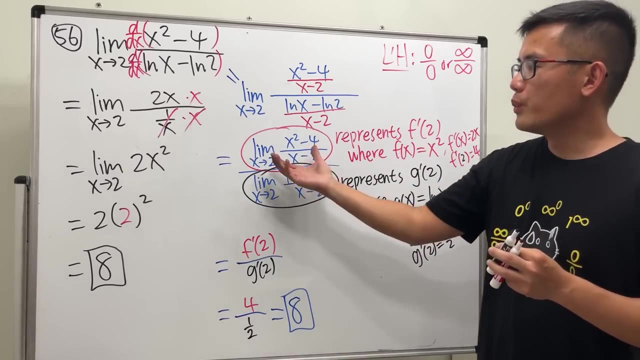 and the reason why there are a lot of mathematicians don't like the Lapito's rule- because it cause circular reasoning- is because you see how when we are doing limits, we are using derivative, but when we are trying to get derivative we will have to use limit. 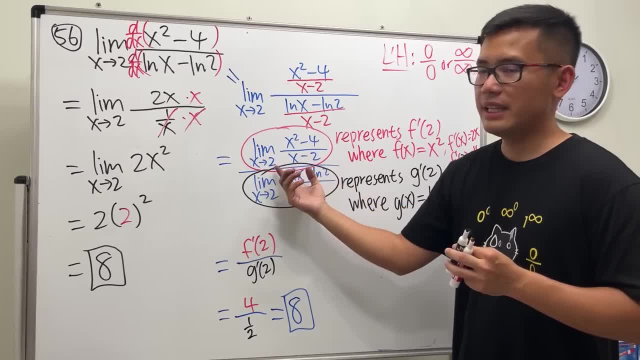 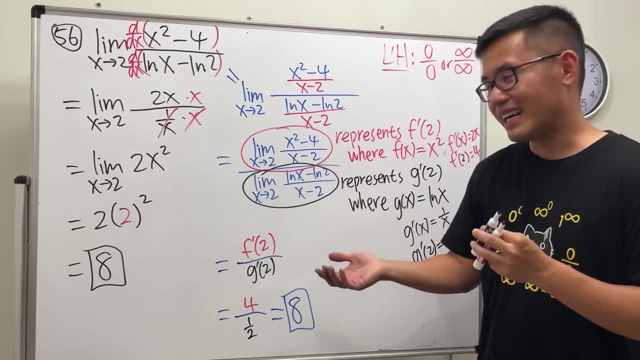 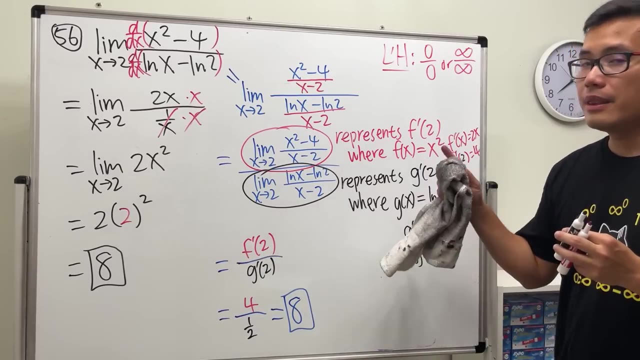 see earlier. when I show you guys this, I cannot just tell you: hey, let's just do the derivative. no, we have to do it algebraically first. yeah, so yeah, be really careful. I will tell you, though, the best time for us to use Lapito's rule is: 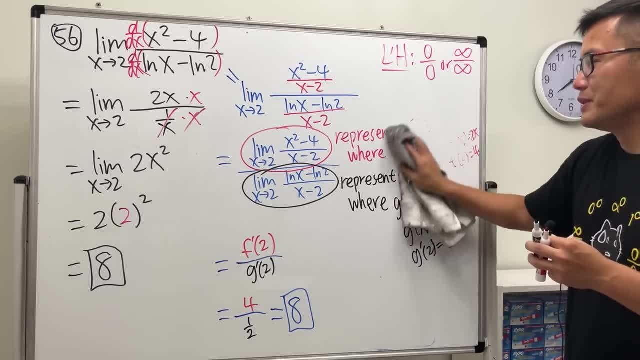 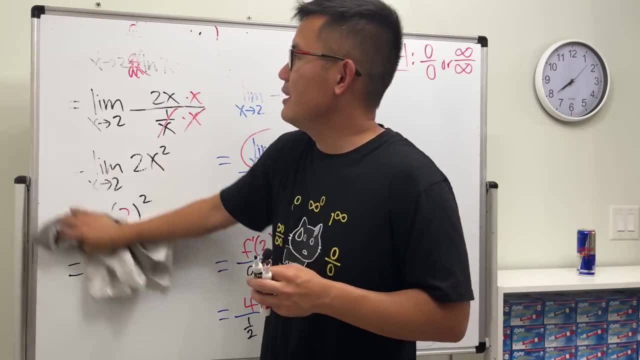 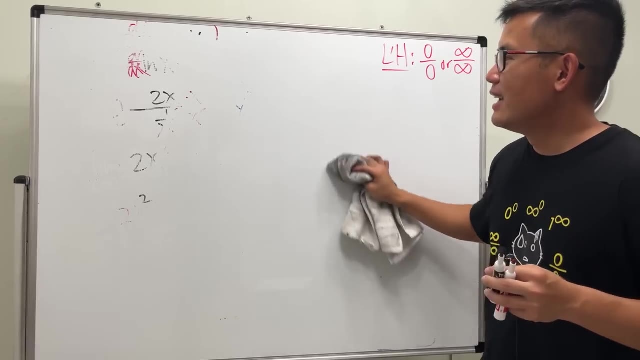 0 over infinity, but then still a lot of people will still not like it too much, but it's convenient. I will say, yeah, that's the explanation, because I want to move on, and usually I will just say I want to go home, but I'm home already, so it's not like. 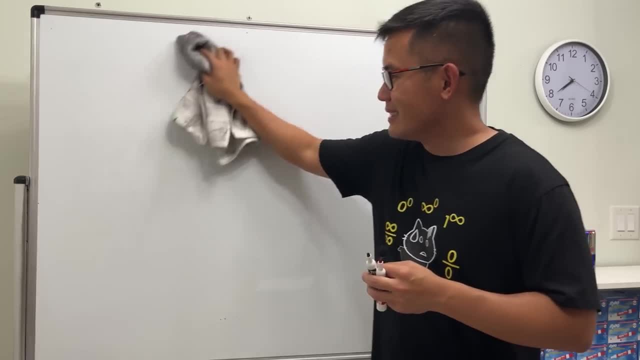 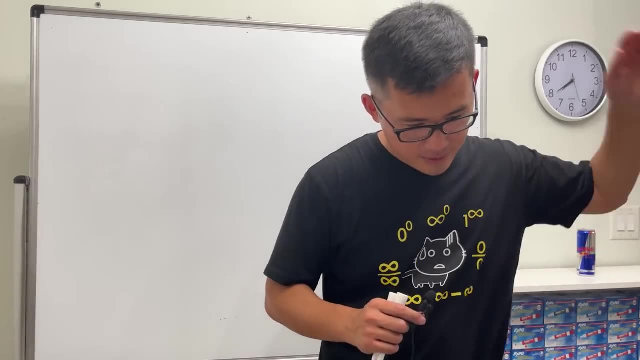 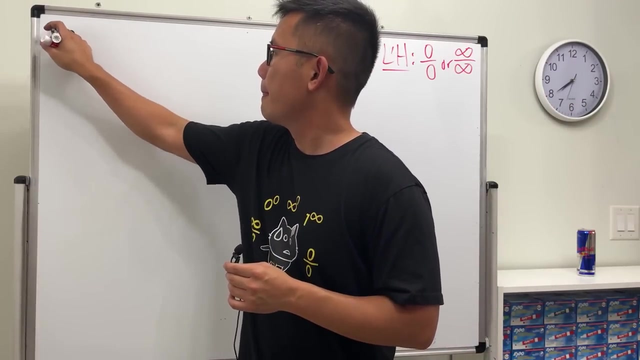 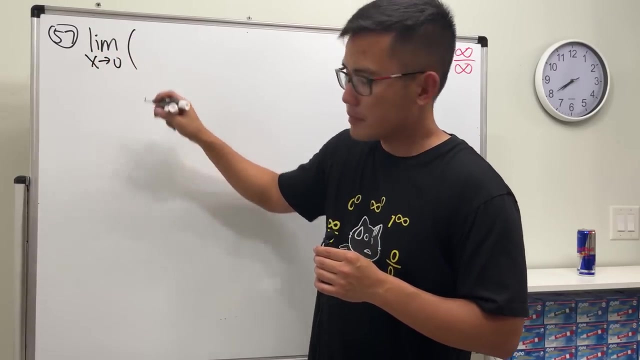 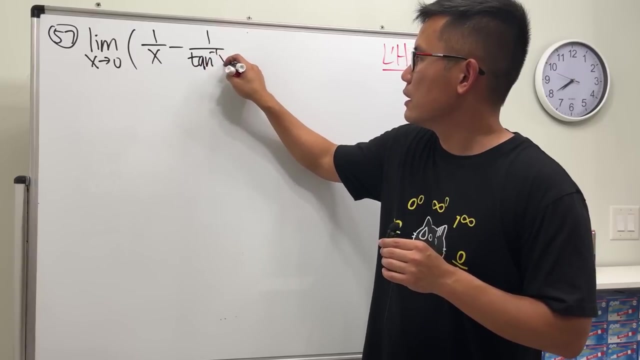 when I was doing that, 100 integral or 100 derivative equations. okay, number 56, no, number 57 limit, give you guys a tough one. x approaching 0, and then we have 1 over x minus 1 over inverse tangent of x. okay, just trust me for this one. 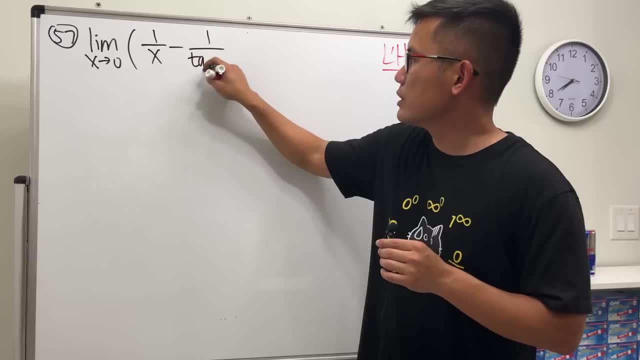 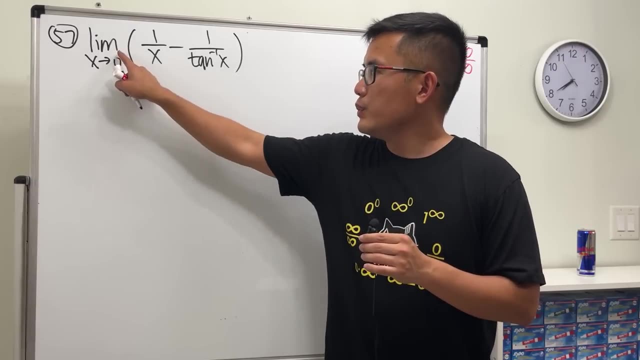 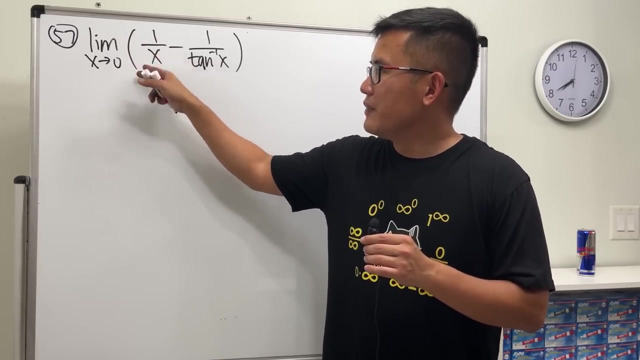 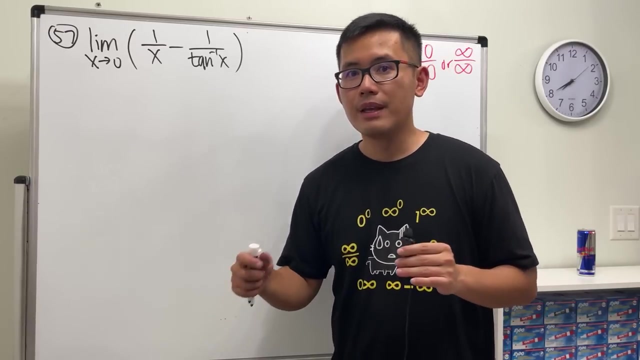 so if yourophilic plus replace by infinity be, the raise is equal to zero. no, zero plus over inverse tangent x. okay, so now this insanity rule is: спасибо for me, minus one over inverse tangent. okay, just trust me for this one. technically we do the zero plus for zero minus, but 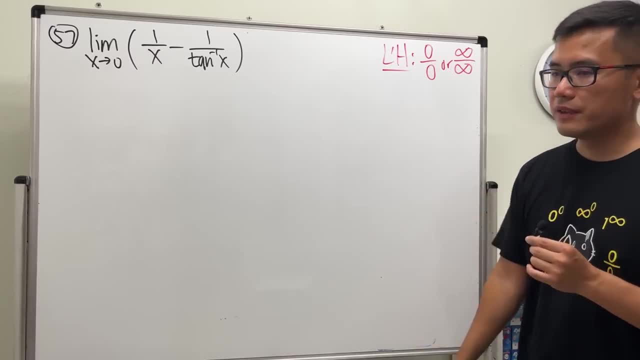 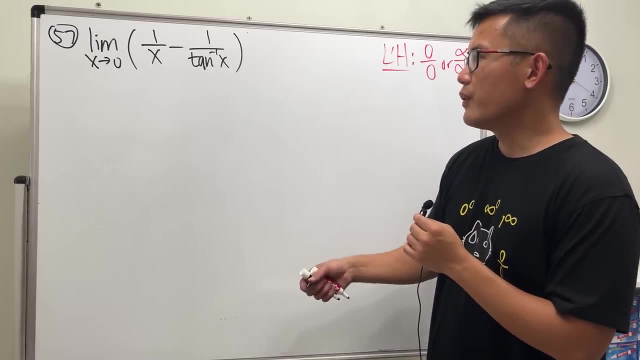 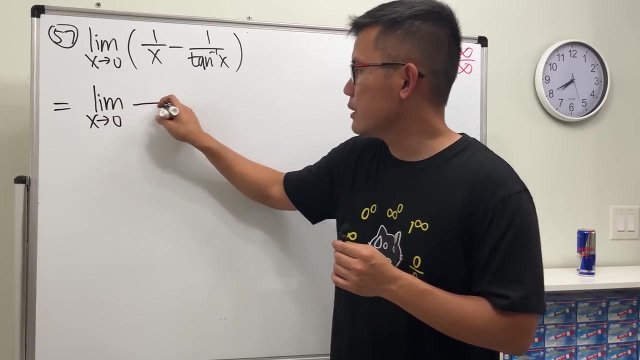 if we have zero plus, we get infinity minus infinity of infinity, namely a fraction. here we have two fractions. not good idea. therefore, let's just combine them and to do so, i'm just going to write this as the limit as x approaching zero, right. we need this and that together, right? so it's x times inverse tangent of x. 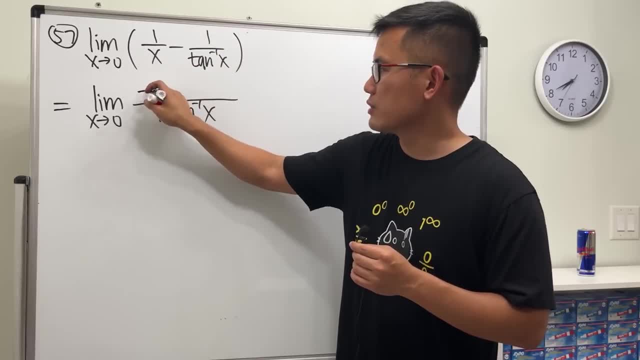 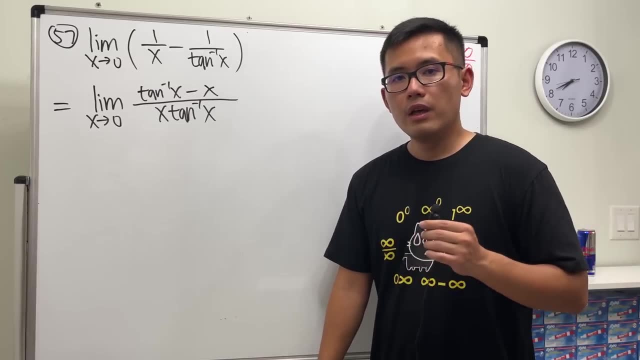 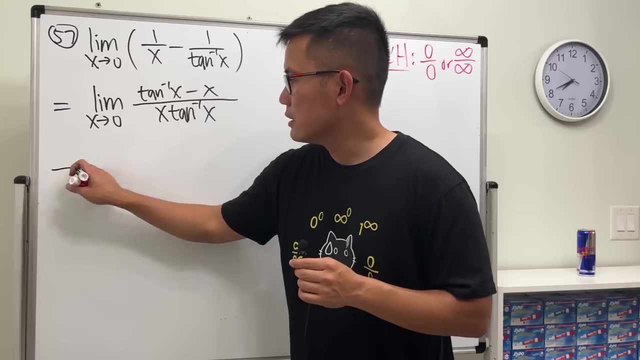 and then pretty much multiply inverse tangent of x here. so we need the inverse tangent of x here and then minus just x there. much better. and you can check if we have zero into all the x's, we get zero over zero and because of that let me just indicate that we have zero over zero. we are using. 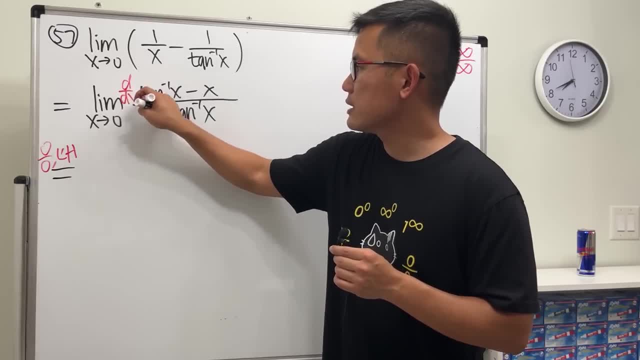 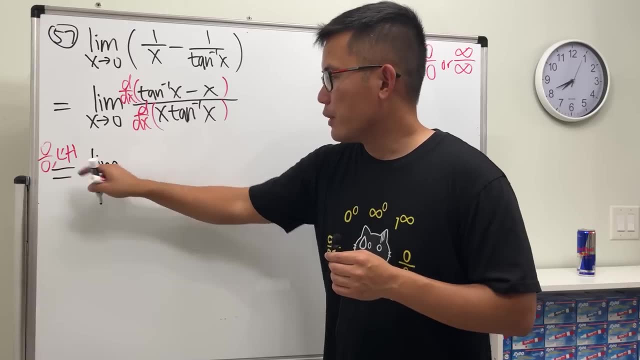 the law of vitals rule. i'm just going to put d? dx and d dx just to show you guys that we are using a so-called law of vitals rule. i forgot to put this earlier, so just go ahead and do it on your go back to your notes. 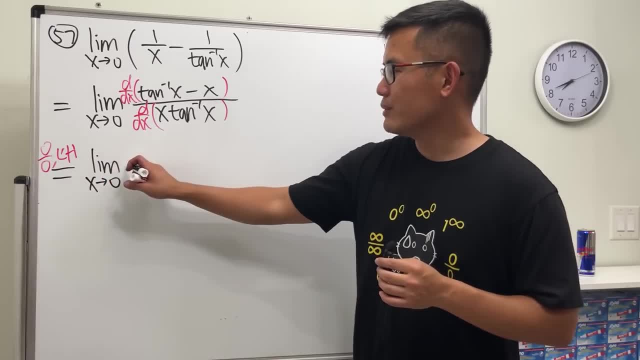 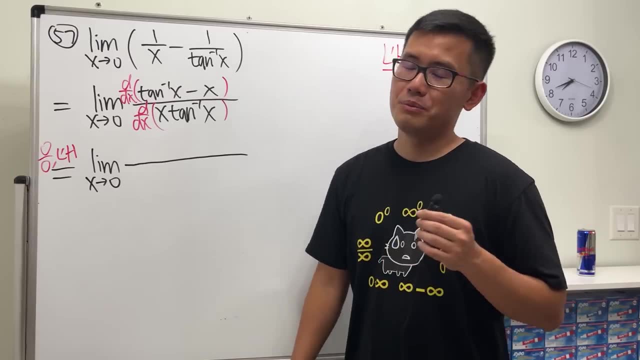 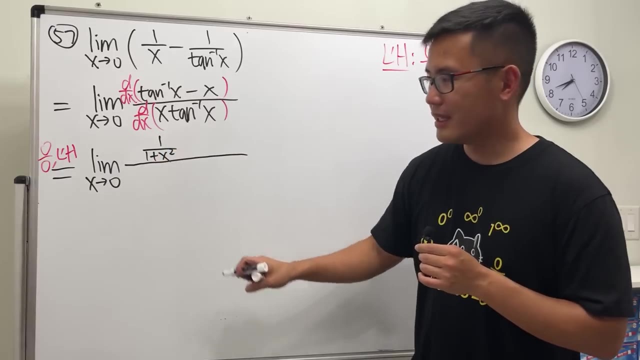 and do it as i told you. you have to know your derivatives really well. what's the derivative inverse tangent of x? do i need to go to the board? sure, but i don't need to because i know the derivative, that is one over one plus x square. okay, the derivative of one. let's see the derivative. 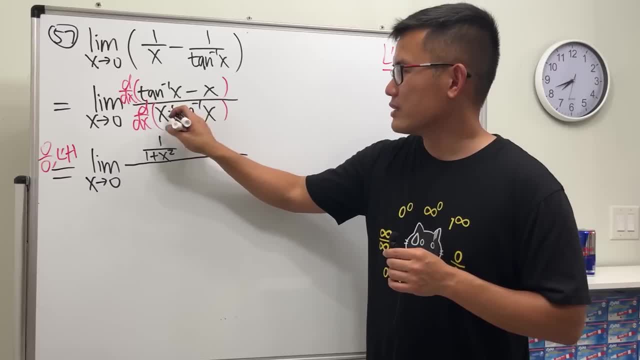 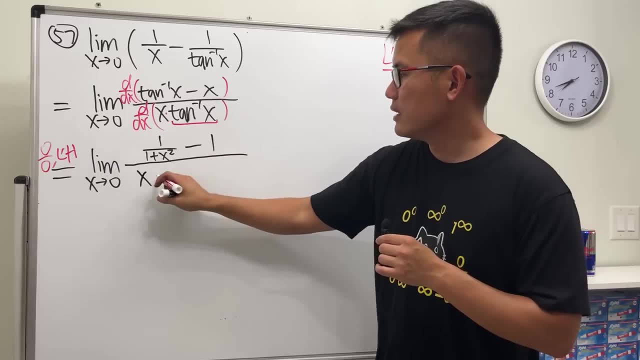 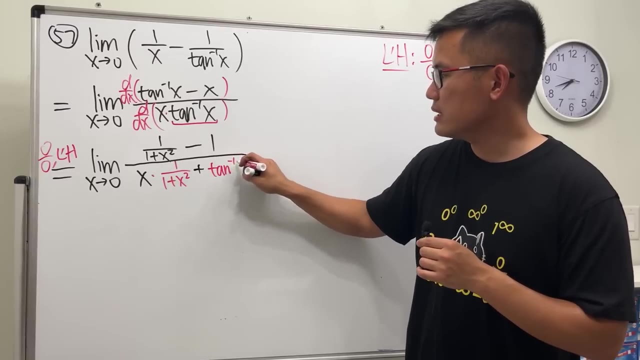 this is one, so it's minus one. this right here we need a so-called product rule. we are going to keep the first function, which is x you, and then times the derivative of the second, so that is one over one plus x square, and then we add the second function, which is inverse tangent of x times the derivative of the first, so it's one. 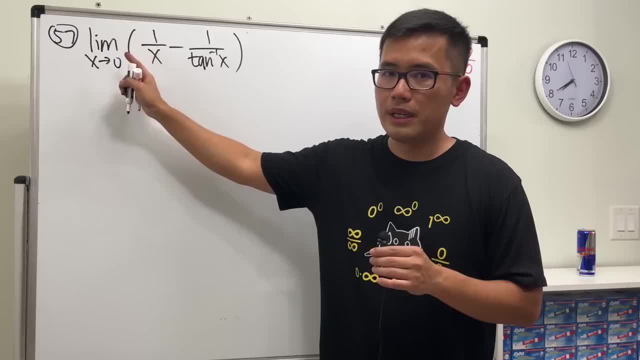 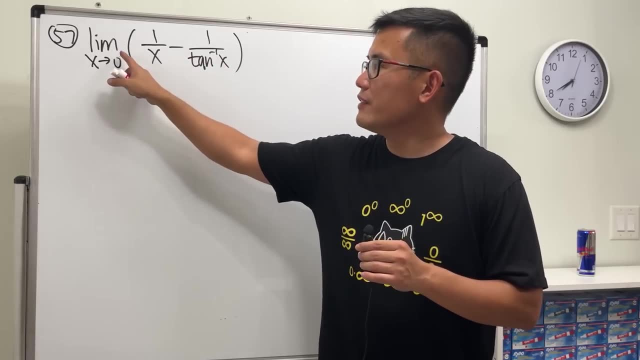 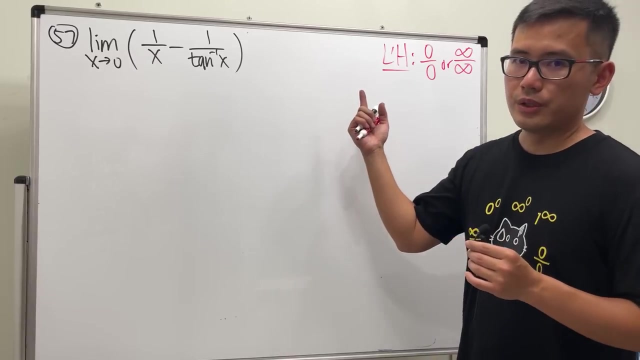 technically, we do the 0 plus or 0 minus. but if we have 0 plus, we get infinity minus infinity. if we have a minus here, we still get infinity minus infinity. so indeterminate point. either way, in order for us to use Lapito's rule, 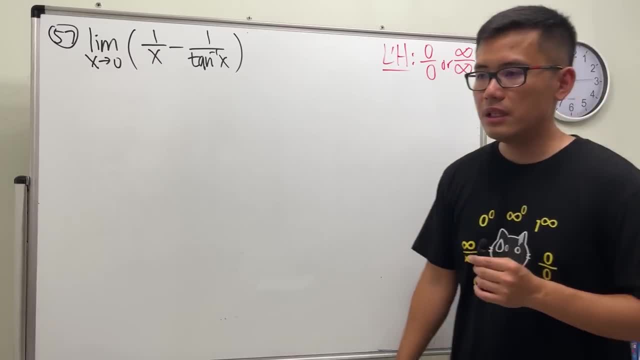 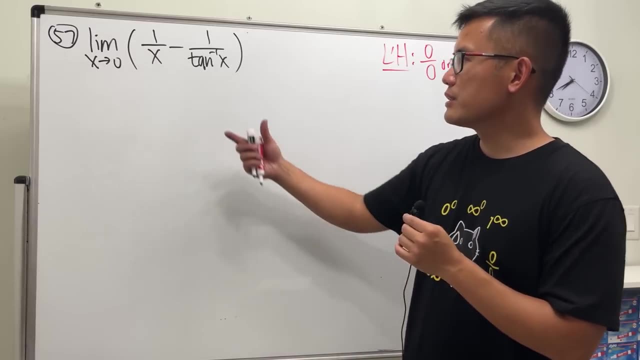 you see that we have to have 0 over 0 or infinity over infinity, namely a fraction. here we have two fractions. not a good idea. therefore, let's just combine them and to do so, I'm just going to write this as the limit, as x of. 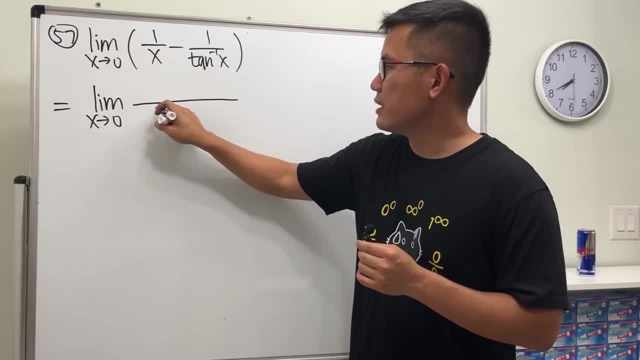 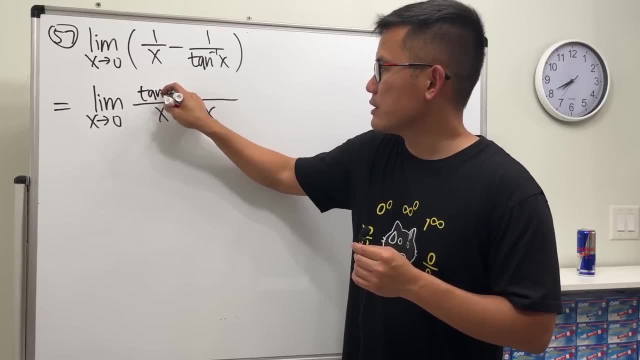 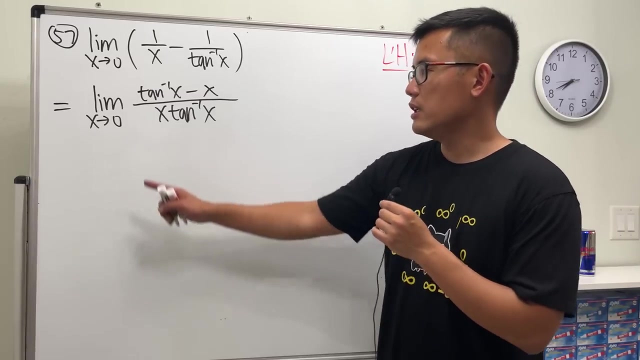 approaching 0. right, we need this and that together right? so it's x times inverse tangent of x and then pretty much multiply inverse tangent of x here. so we need the inverse tangent of x here and then minus just x there. much better and you can check if we. 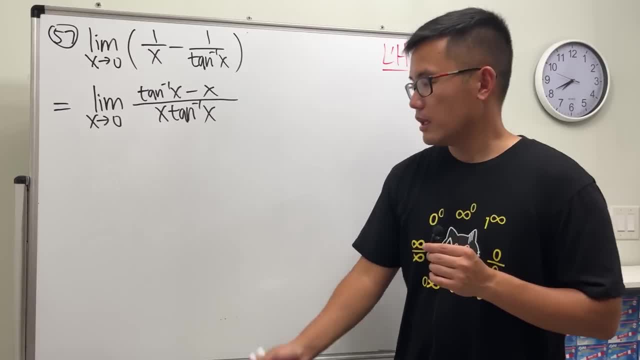 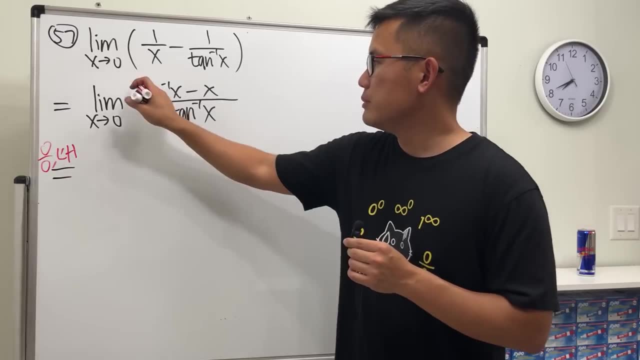 have 0 into all the x's, we get 0 over 0 and because of that, let me just indicate that we have 0 over 0. we are using the Lapito's rule. I'm just going to put x and d dx just to show. 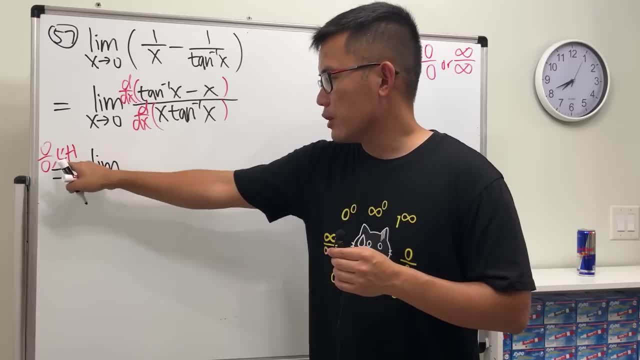 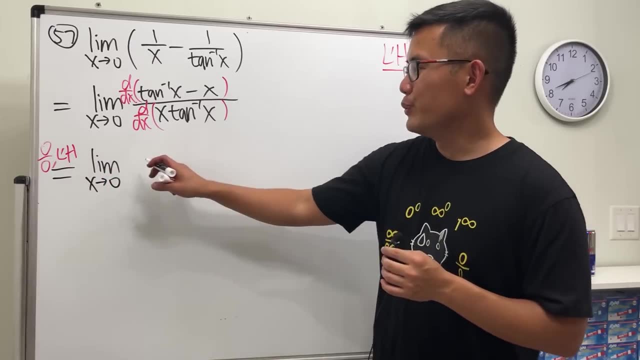 you guys that we are using the so called Lapito's rule. I forgot to put this earlier, so just go ahead and do it on your own. go back to your notes and do it as I told you. you have to know your derivatives really well. what's the derivative inverse tangent of x? 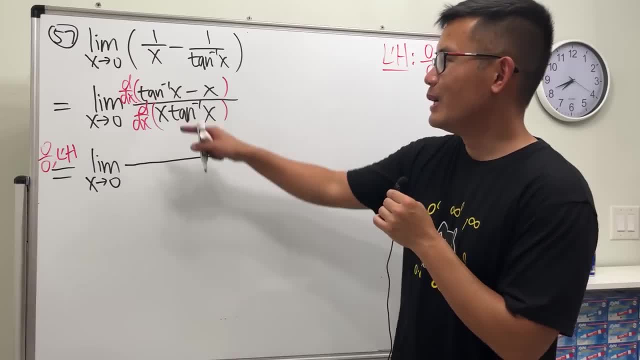 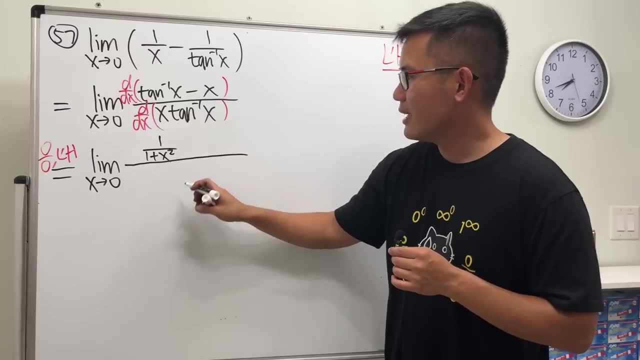 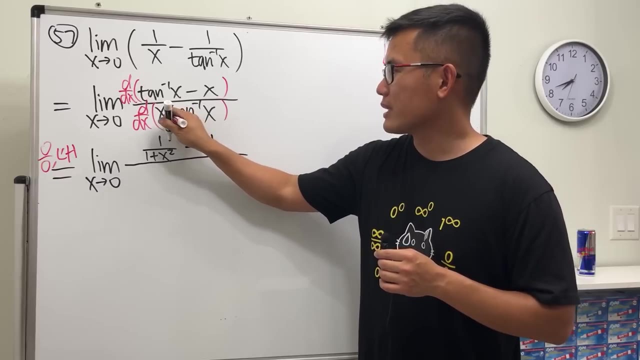 do I need to go to the board? sure, but I don't need to because I know the derivative that is 1 over 1 plus x squared. okay, derivative of 1. derivative of this is 1, so it's minus 1. this, right here we need the so called product rule. 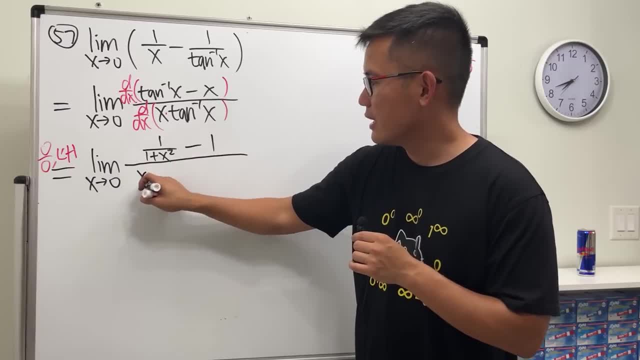 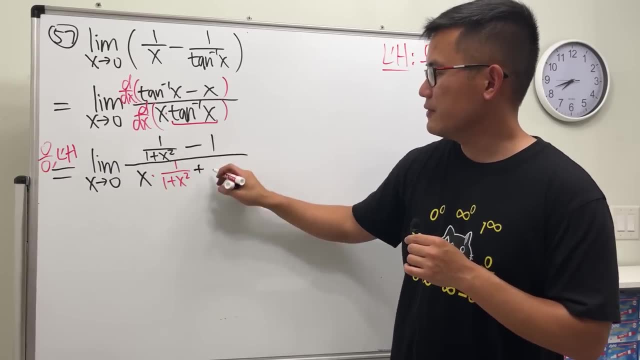 we are going to keep the first function, which is x, and then times the derivative of the second, so that is 1 over 1 plus x squared. and then we add the second function, which is inverse tangent of x times the derivative of the first, so it's 1. 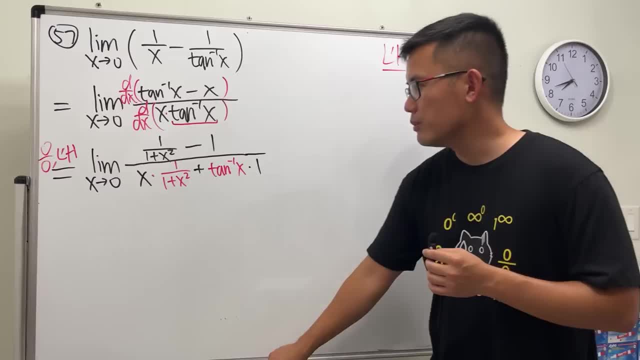 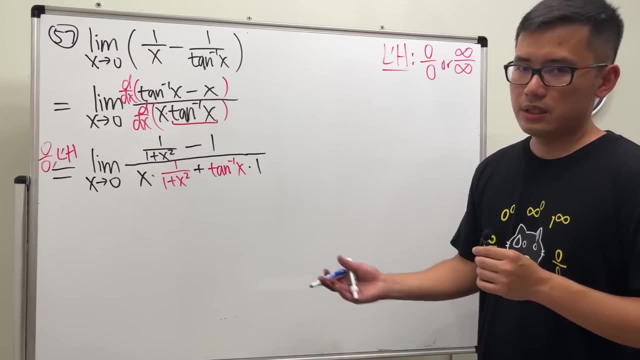 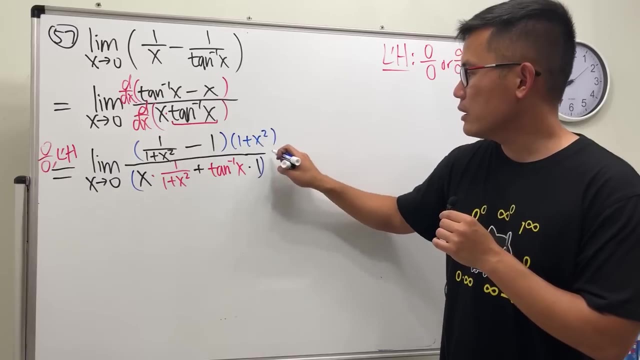 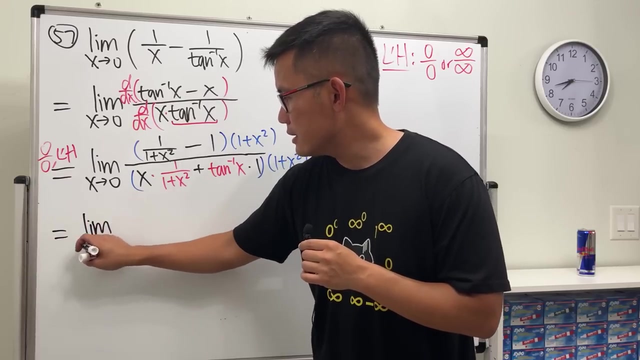 so these are the things that you would need to be able to do for your derivatives before we proceed. let's fix the complex fraction situation, and that is to multiply the top and bottom by one plus x square, and likewise here. so let's see, we will have limit as x approaching zero. this times that is just one. 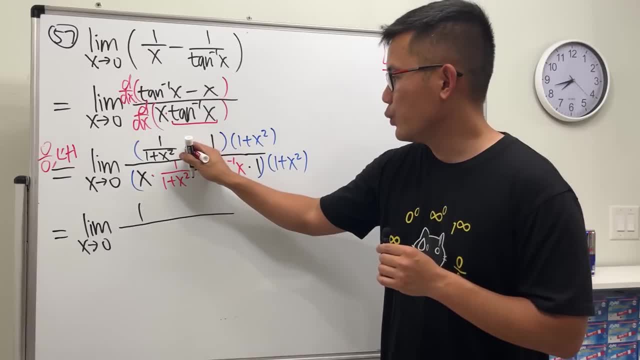 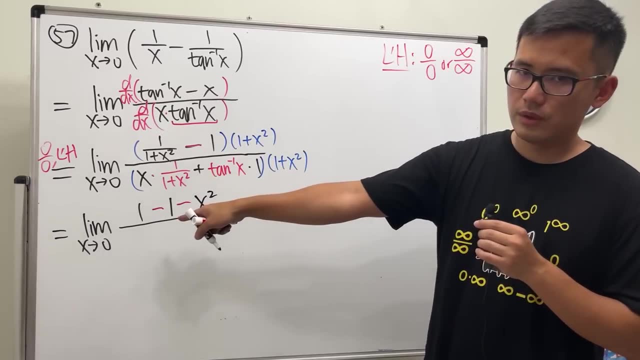 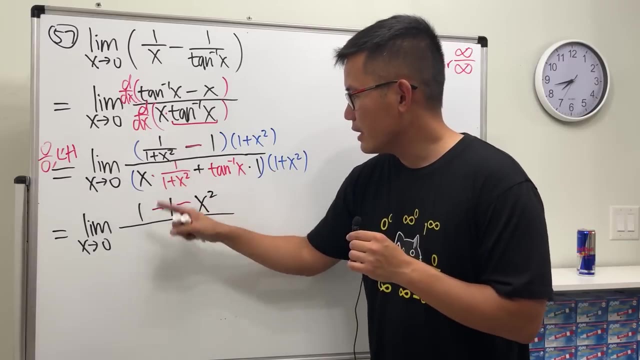 this times that let's distribute the negative. so we will have negative one and then minus x square. that's cool. we have the one minus one. so far, so good. i don't know. anyway, take this times that the one plus x cancel. so we just do it like this and then we have the one minus x square. 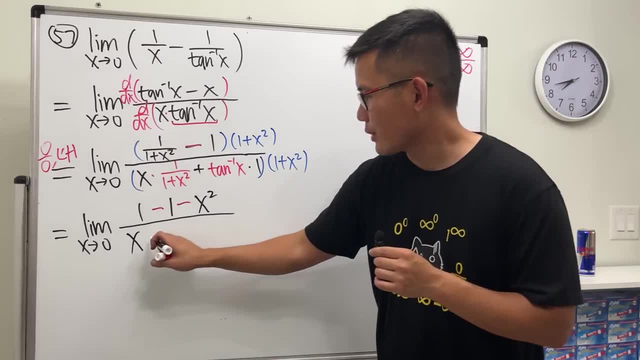 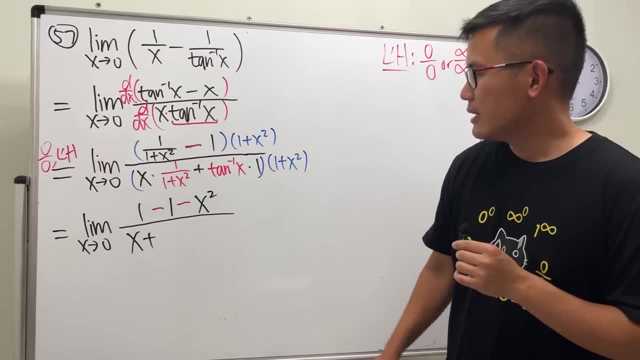 and then we have the one minus x square. so we get the one plus x square plus one minus x square, and then we just now consider that reverse tangent and we just add it, and then we have to find the positive sign and we do the fourth problem. this is the negative, so this should have x this times. 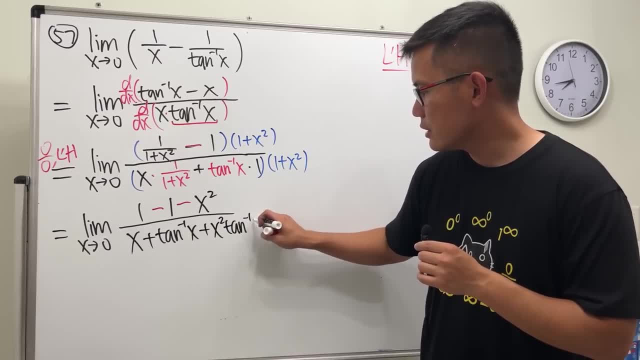 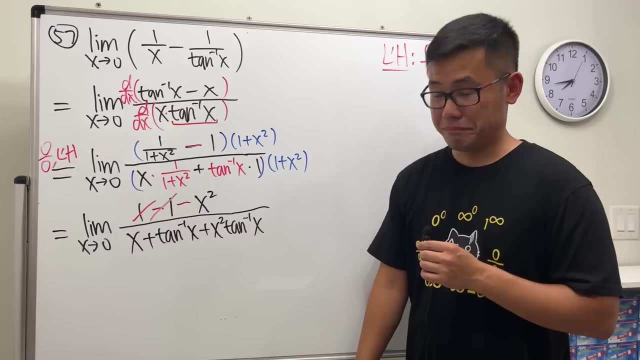 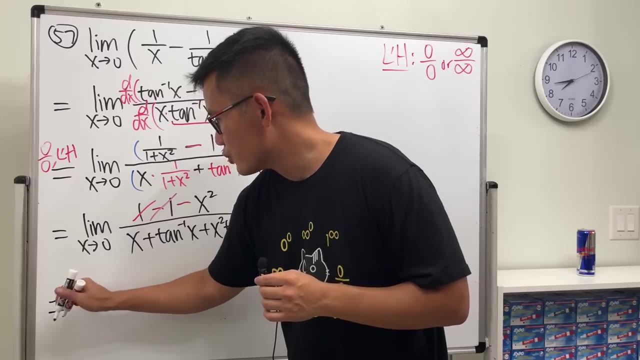 ah, okay, plus, let's, let's distribute, so this times the infrostantion of x, and then this times that. so it's plus x square inverse tangents of x. i told you this is a hard one, but anyway, one minus one, zero over zero. so, yes, do lapito's rule again. try it, it is making us progress. oh yeah, so here we go. 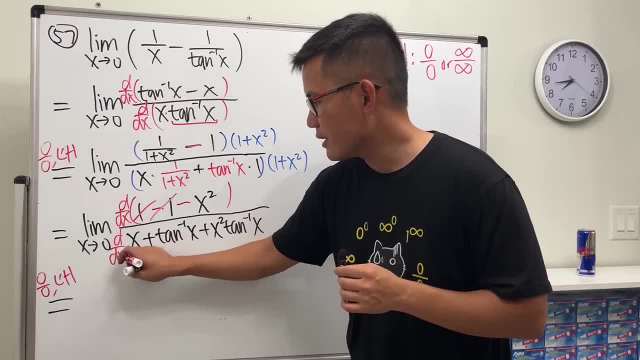 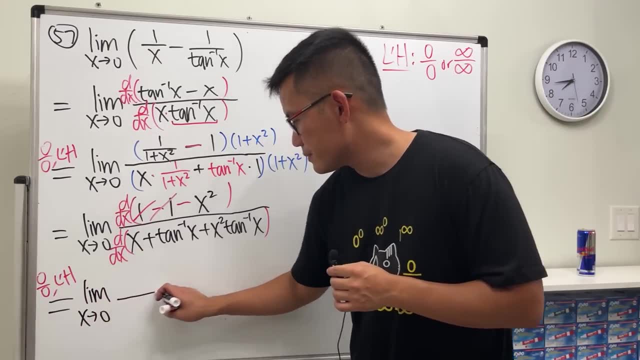 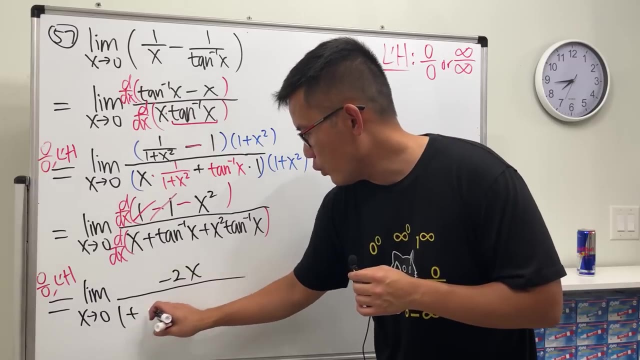 lapito's rule on the top, differentiating on the top, and then take the derivative on the top on the bottom limit as x approaching zero, the derivative of this guy is negative 2x derivative. x is 1 derivative. this is 1 over 1 plus x square derivative. this product rule again. 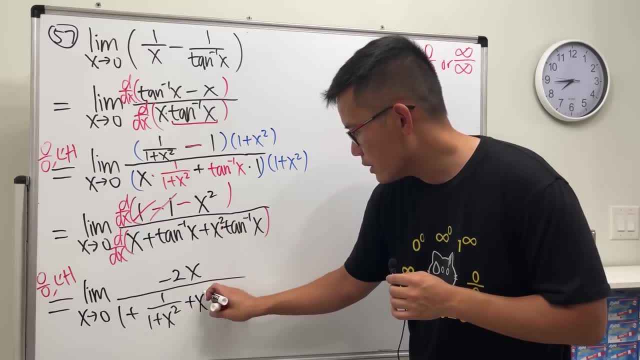 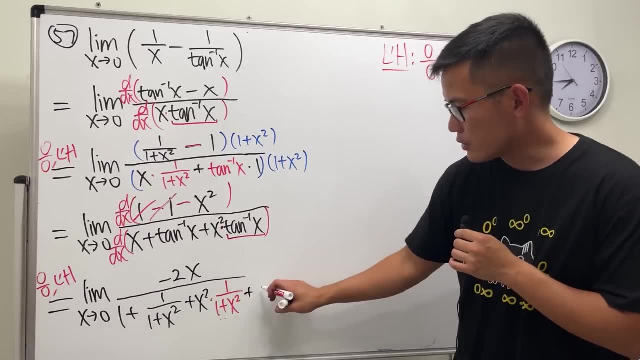 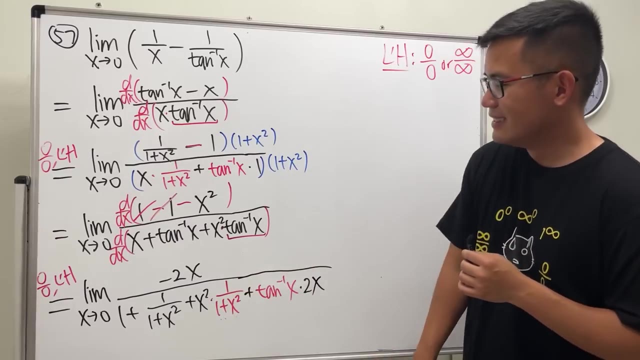 the first function is x square times the derivative of the second, which is 1 over 1 plus x square. and then we add the second function, which is inverse tangent of x times the derivative of the first, which is 2x. i know sometimes you want to do the derivative. 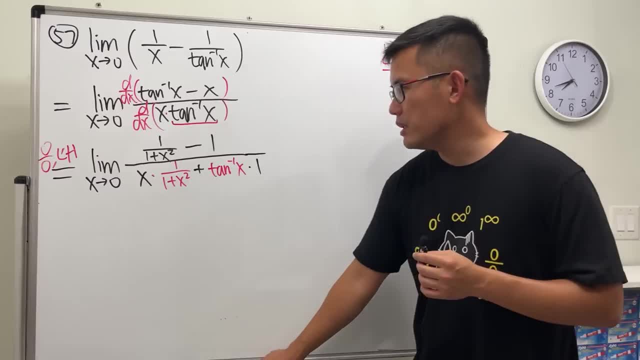 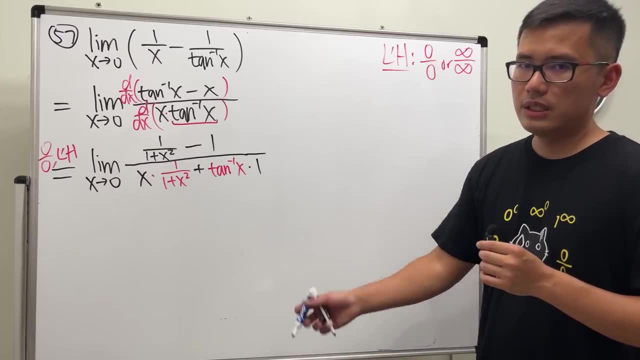 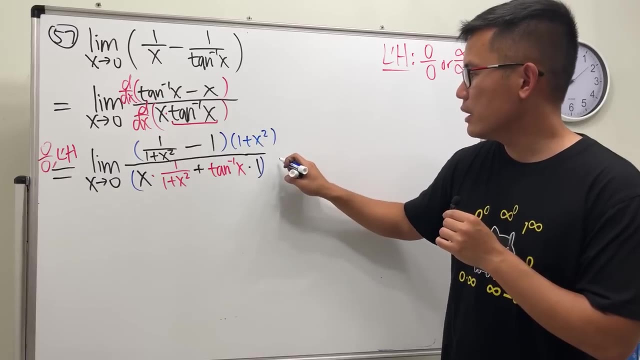 so these are the things that you would need to be able to do for your derivative. before we proceed, let's fix the complex fraction situation, and that is to multiply the top and bottom by 1 plus x squared, and likewise here. so let's see we will have 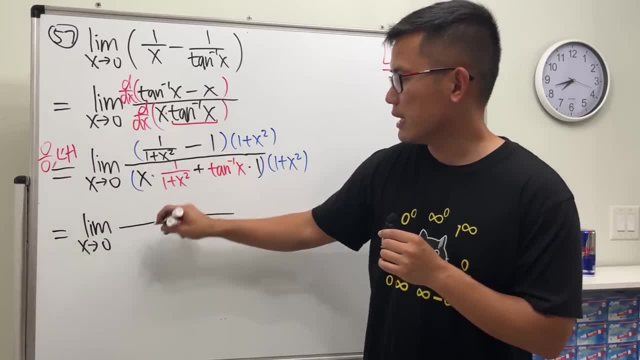 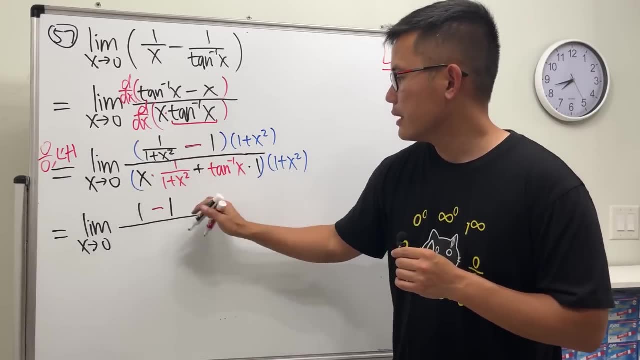 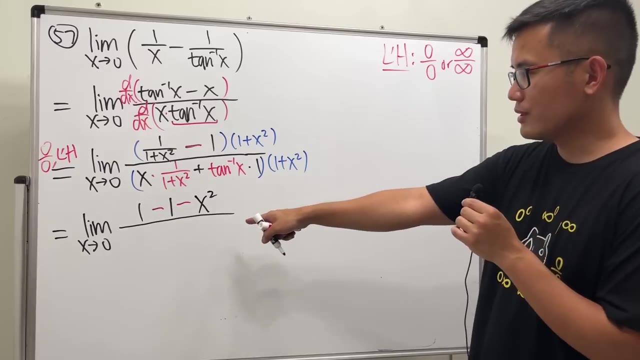 limit as x approaching 0. this times, that is just 1. this times that let's distribute the negative, so we will have negative 1 and then minus x squared. that's cool. we have the 1 minus 1. so far, so good. anyway, take this: 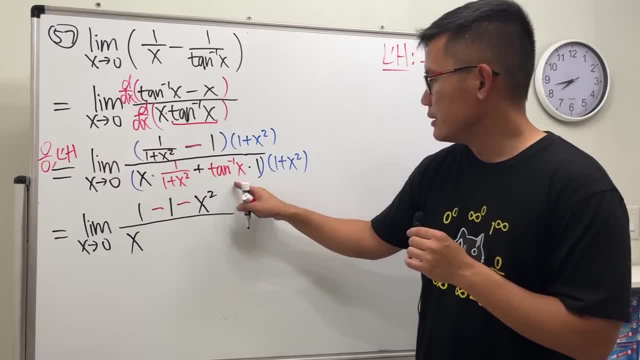 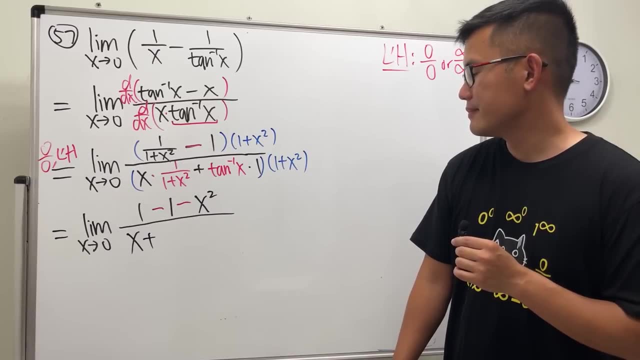 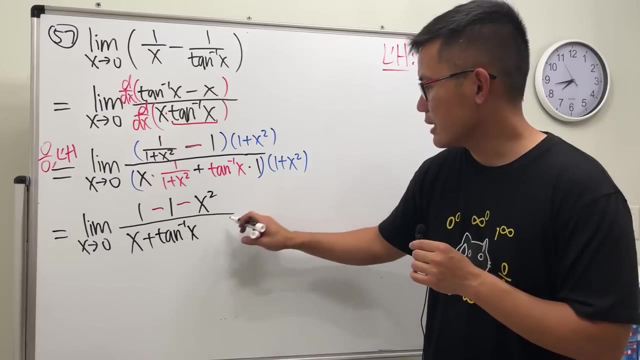 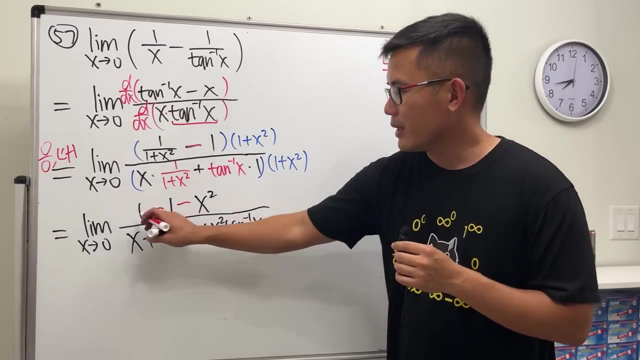 times that the 1 plus x cancels, so we just have x. this times that plus, let's distribute. so this times that is inverse tangent of x and then this times that plus x squared, inverse tangent of x. I told you this is a hard one, but anyway. 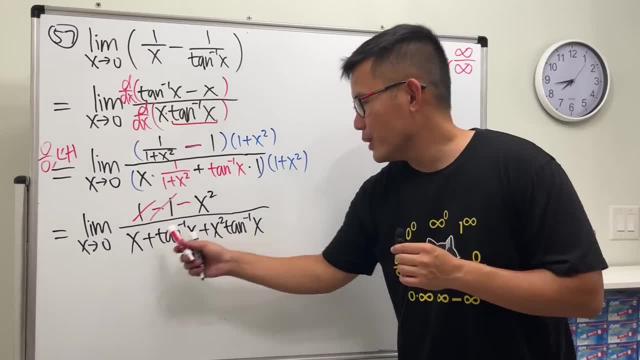 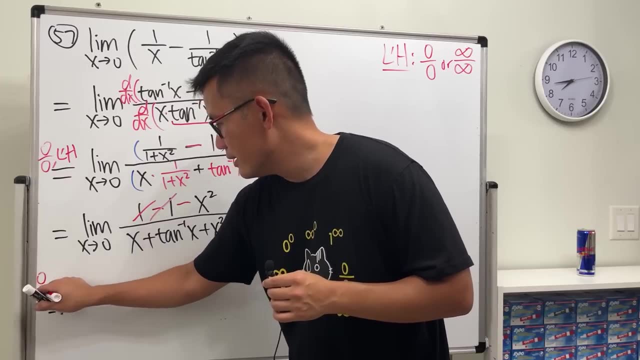 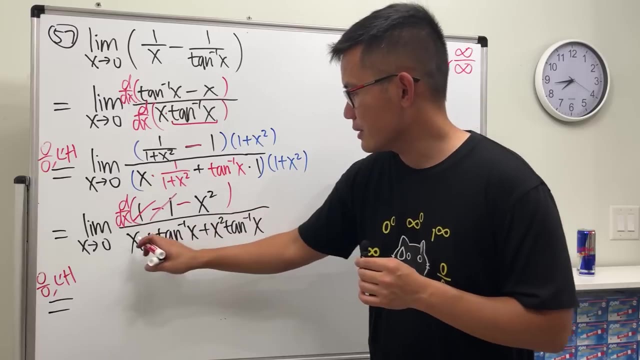 1 minus 1 is 0. plugging 0 into all the x's, I tell you, is 0 over 0. so yes, do Lapito's rule again. try it. it is making us progress. yeah, so here we go. Lapito's rule on the top. 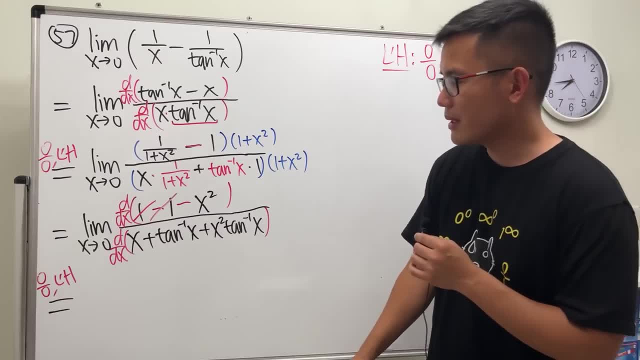 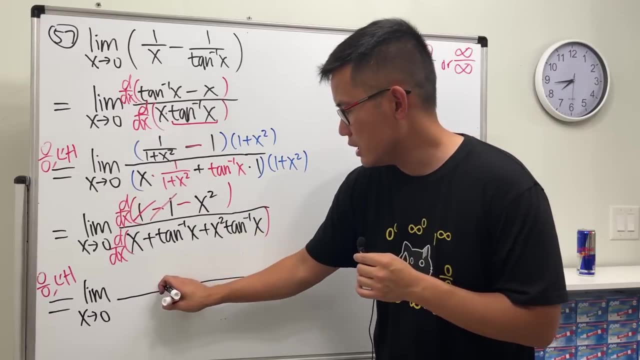 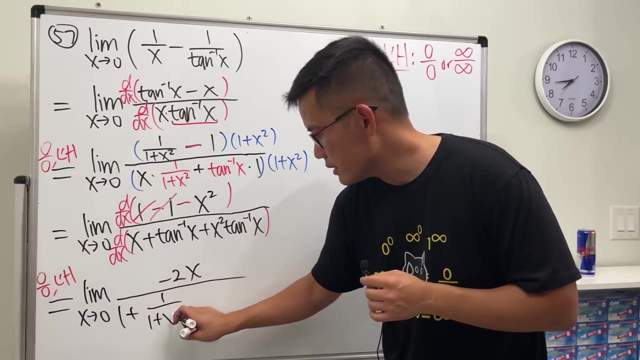 differentiating on the top and take the derivative on the top on the bottom limit, as x approaching 0, derivative of this guy is negative. 2x derivative of x is 1. derivative of this is 1 over 1 plus x squared. derivative of this: 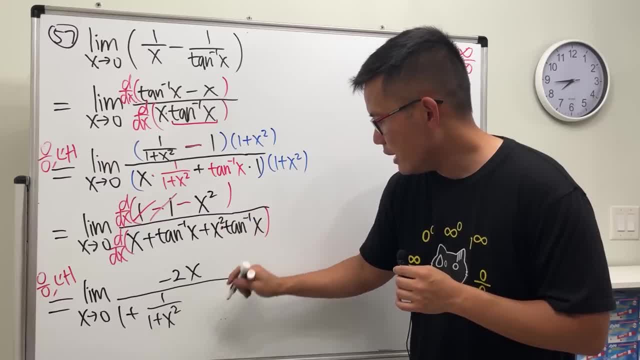 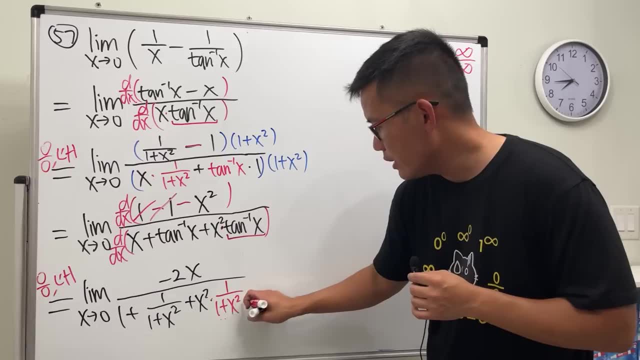 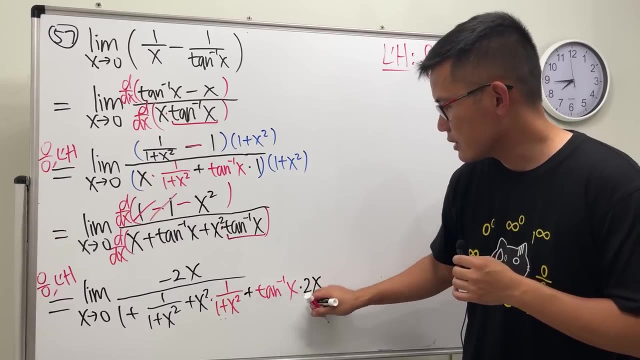 Prata rule. again, the first function is x squared times the derivative of the second, which is 1 over 1 plus x squared. and then we add the second function, which is inverse tangent of x times the derivative of the first, which is 2x. I know sometimes you want to do the 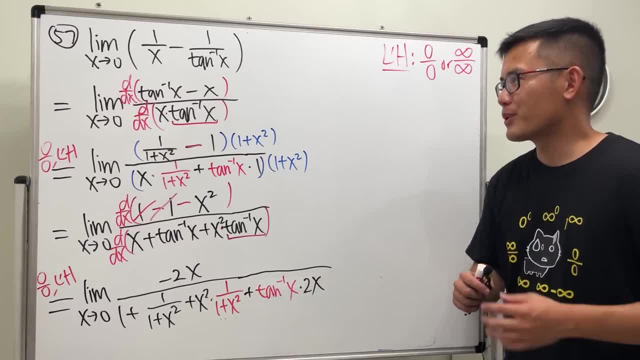 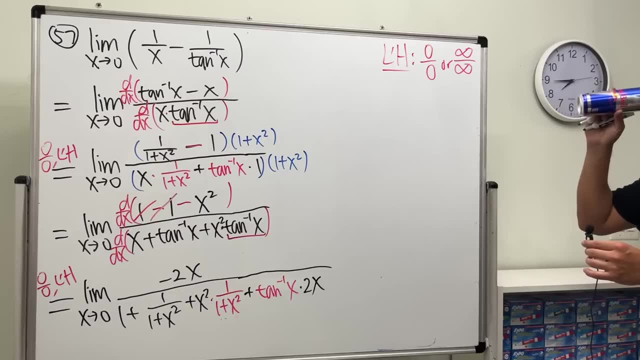 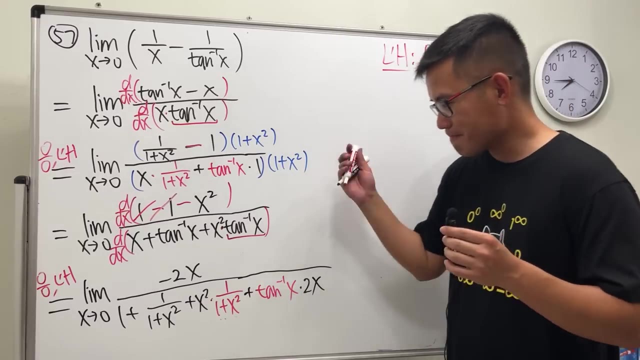 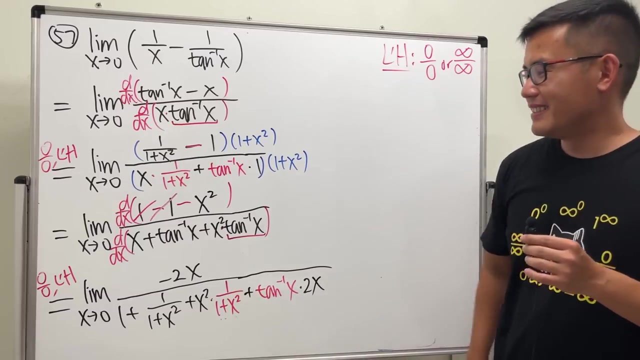 derivatives. Lapito's rule might make you cry, make you want to cry, right? so yeah, if Ripple can sponsor me one day, well, I'll be really happy- or any kind of any like beverage- it doesn't have to be energy drink, anyway. what do we do next? 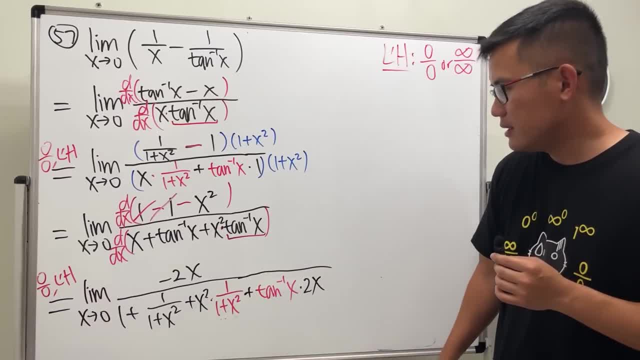 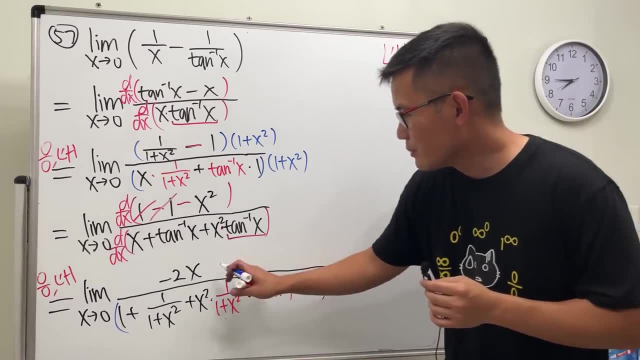 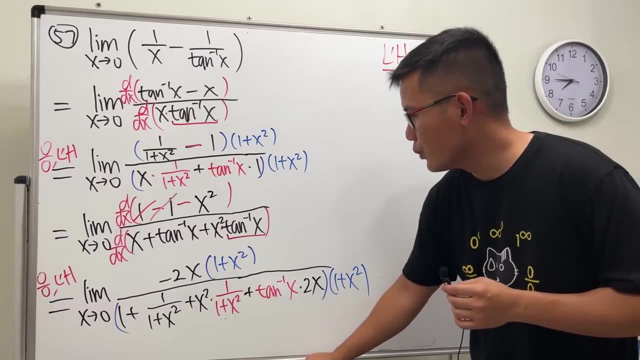 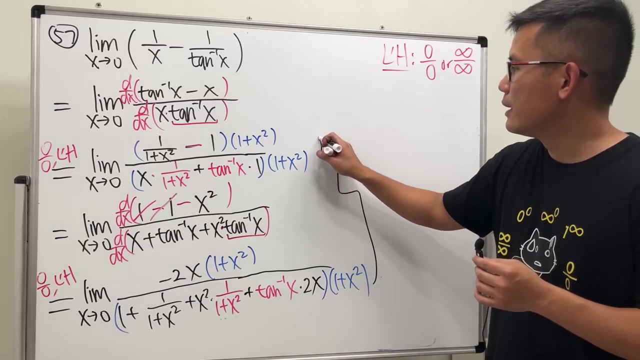 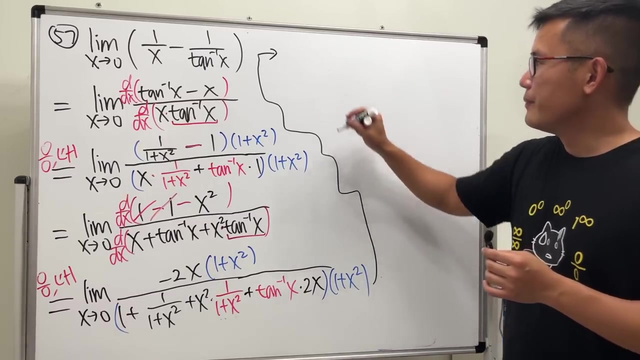 man. okay, let's see this right here. shouldn't be too hard, because I did it before. let's multiply the top and bottom by 1 plus x, squared again, okay. so how am I going to? this doesn't make sense, does it make sense? okay, let's see. 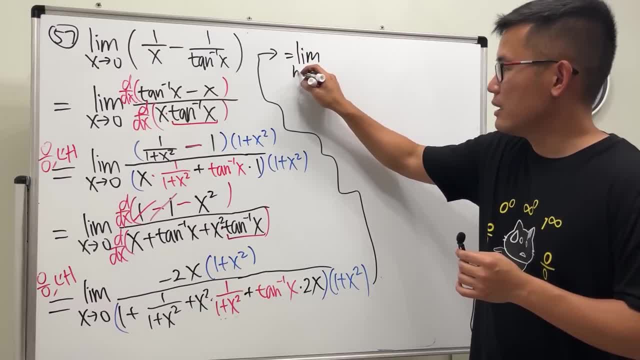 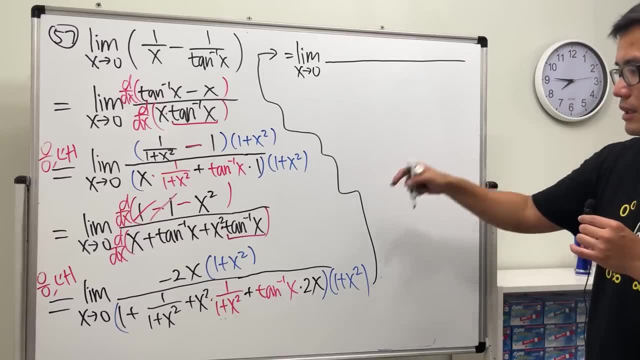 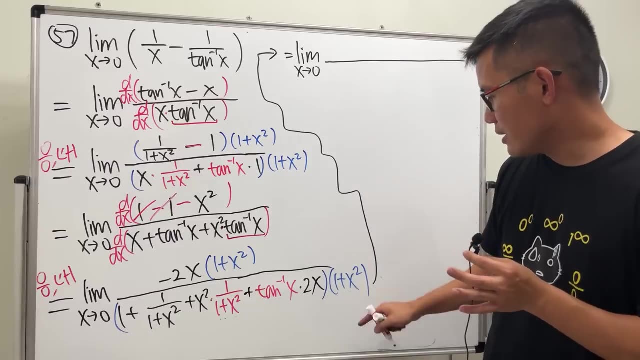 here we have, the limit is x, x approaching 0. perhaps let's multiply the bottom here and see what happens. so before we go there, let's see: this times that we get 1 plus x squared. this times that we get 1 plus x squared. this times that we just get plus 1. 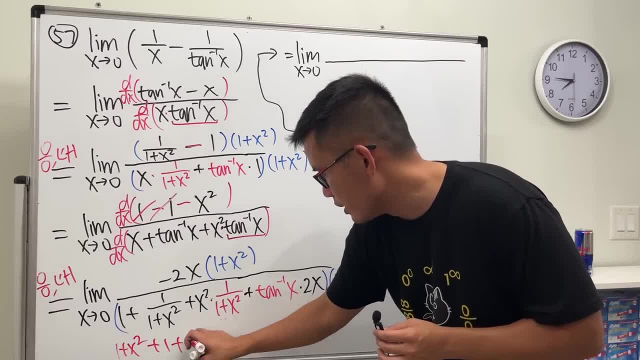 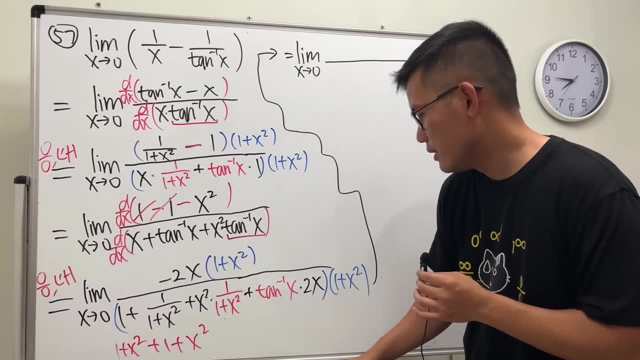 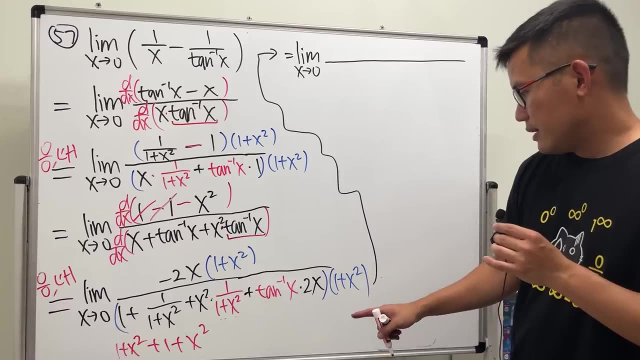 this times that they cancel so we just get plus x squared here, right, and this times that, oh, my god, oh, I don't think we end up with, I don't think we end up with 0 first rule anymore. check this out here: this times, this is just. 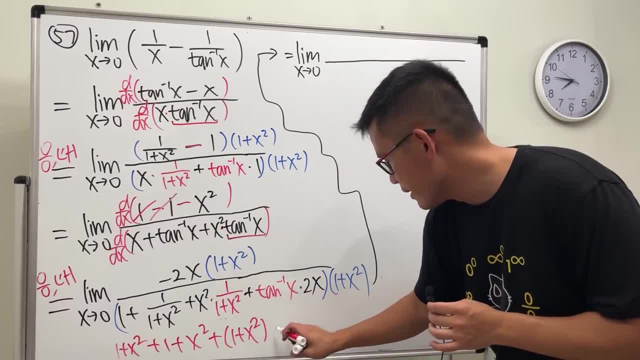 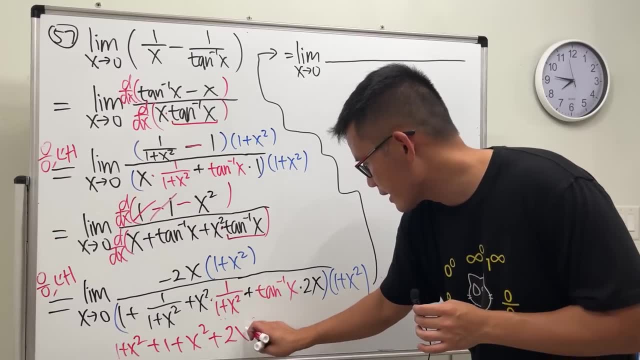 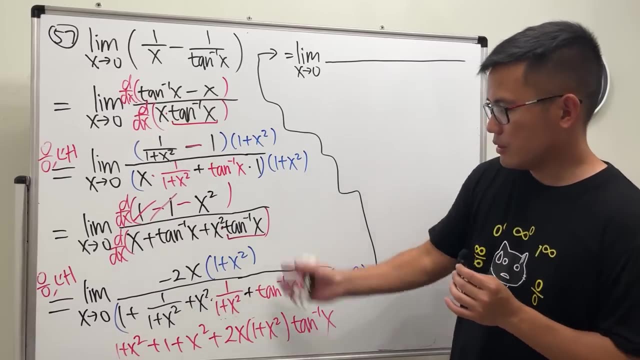 I'm just going to keep it 1 plus x squared, and then let's put a 2x here at the front, first 2x, and then 1 plus x squared at the inverse tangent of x, right, so just multiply it out. the reason that I say it's: 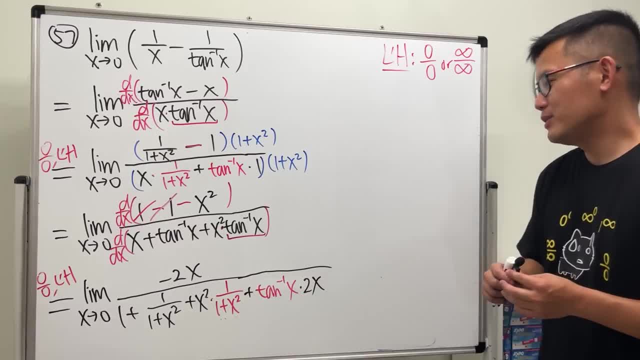 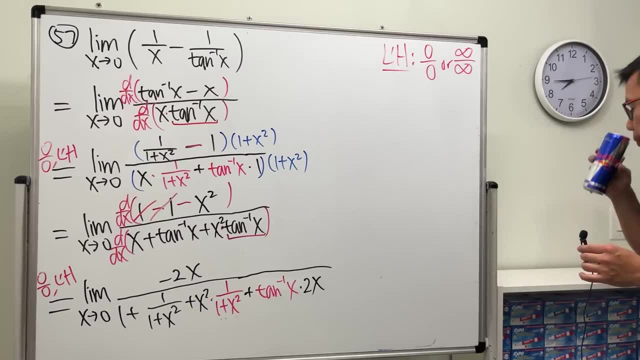 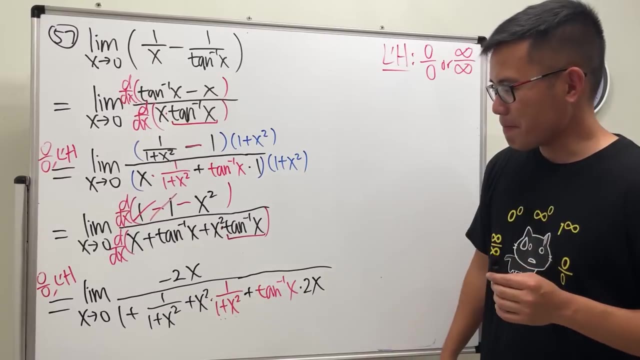 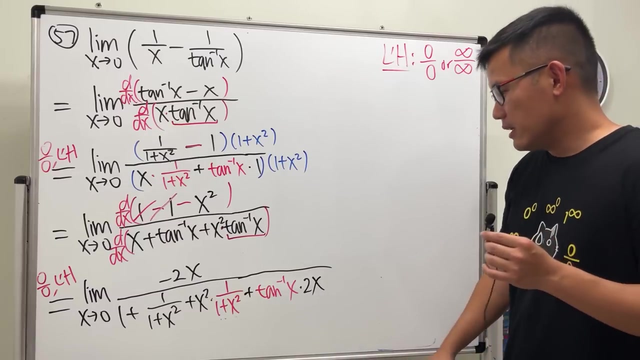 is that? because it might make you cry, make you want to cry, right? so yeah, if ripple can sponsor me one day, well, i'll be really happy- or any kind of any like a beverage- it doesn't have to be energy drink, anyway. what do we do next? man, okay. 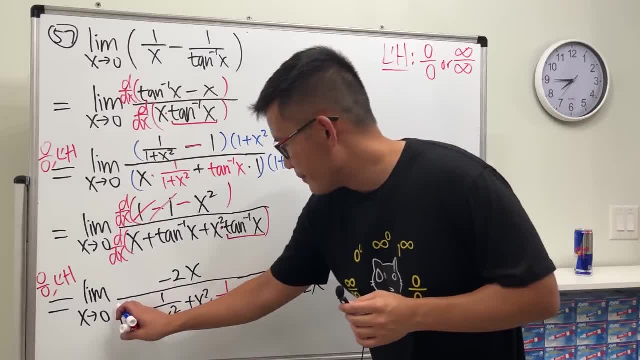 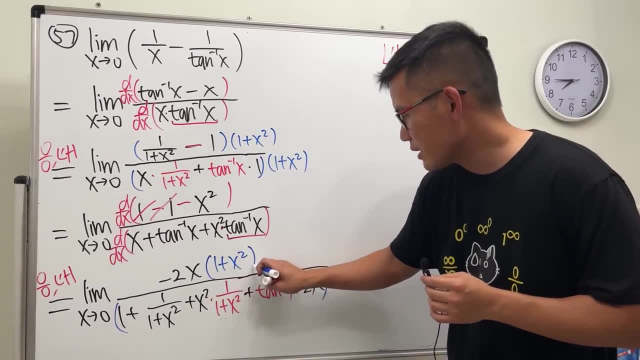 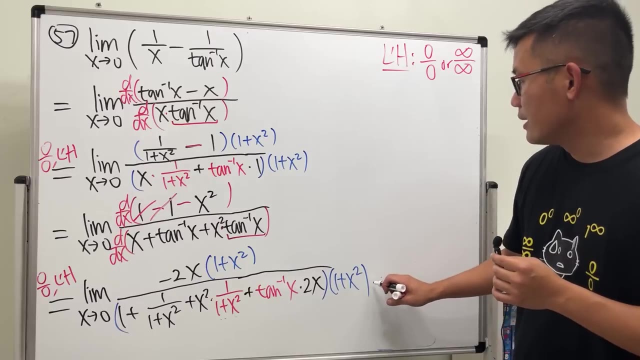 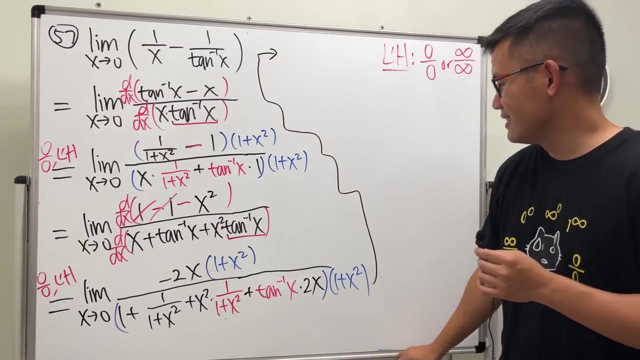 let's see this right here. shouldn't be too hard, because i did it before. let's multiply the top and bottom by 1 plus x, squared again, oh okay. so how am i going to? this doesn't make sense, does it make sense? okay, let's see, here we have. 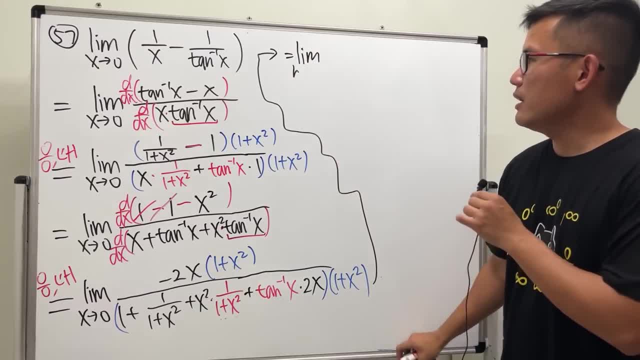 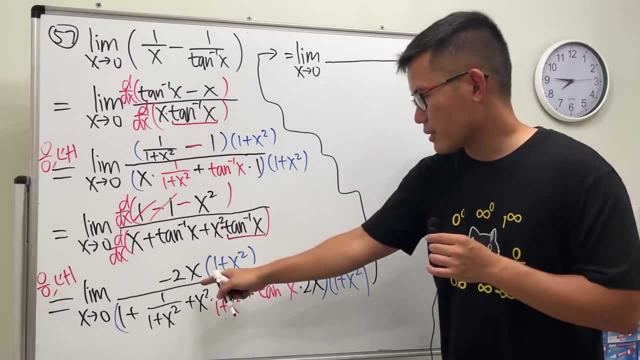 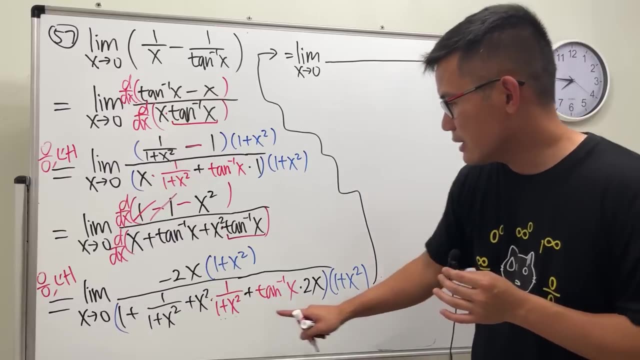 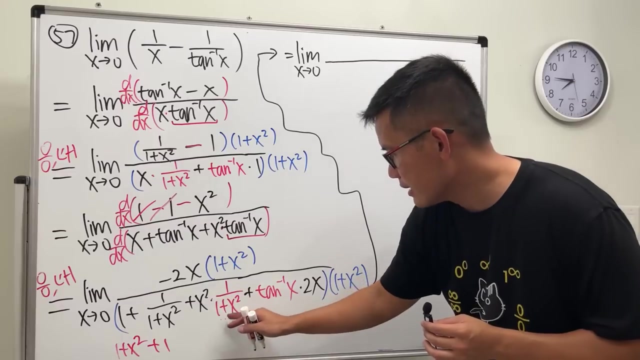 the limit, as you know: x, h, x approaching zero. perhaps let's multiply the bottom here and see what happens, right? so before we go there, let's see: this times that we get 1 plus x squared, this times that we just get plus 1.. this times that they cancel, so we just get plus x squared. 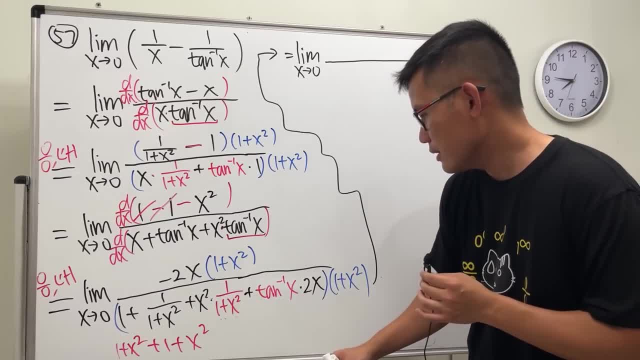 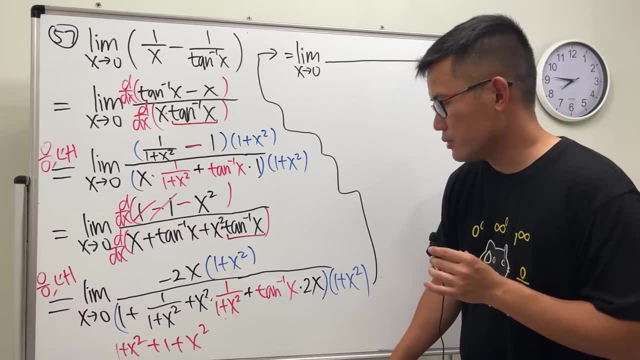 here, right, and this times that, oh my gosh. But oh, I don't think we end up with, I don't think we end up with 0 of s root anymore. Check this out Here: this times, this is just. I'm just going to keep it. 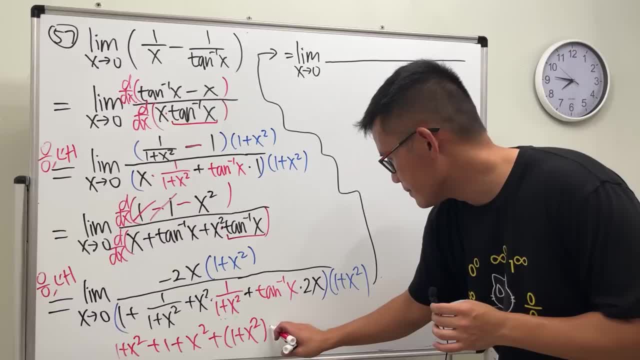 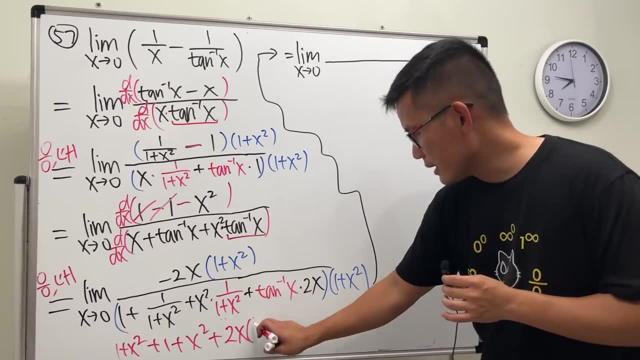 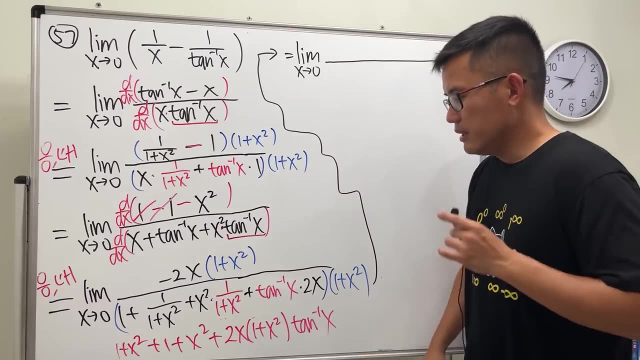 1 plus x squared. and then let's put a 2x here at the front. first 2x, and then 1 plus x squared at the inverse tangent of x. Alright, so just multiply it out. The reason that I say it's not 0 for 0 is because when x is approaching 0,. 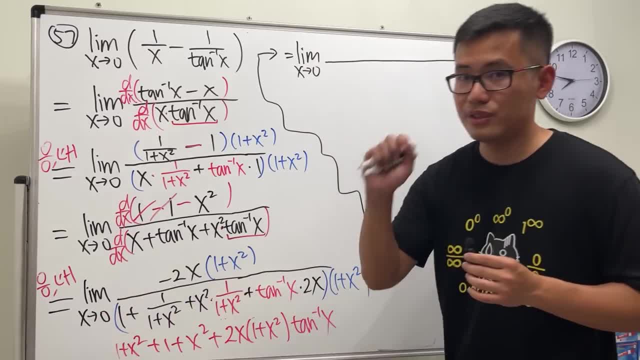 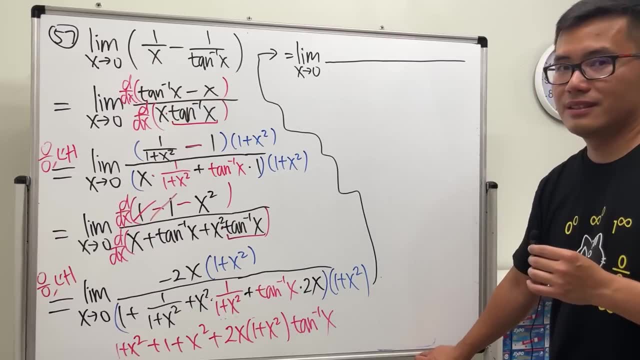 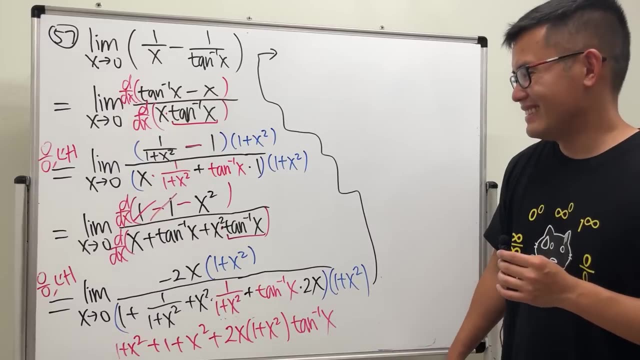 this is 0,. this is 0,, this is 0, but we have 1 plus 1, which is 2 on the bottom, And- but this is upsetting, Because when we put 0 on the top, we get 0.. 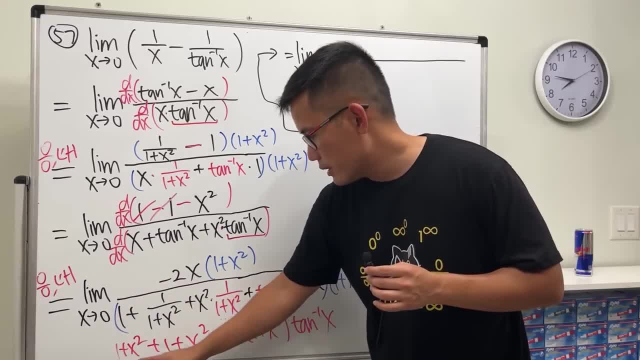 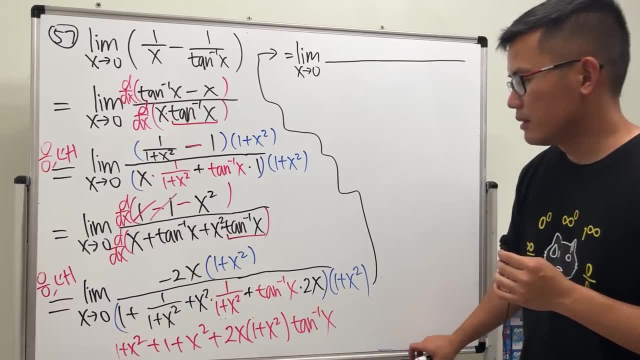 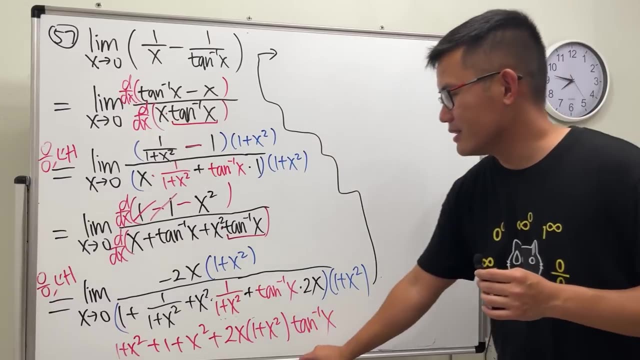 not 0 for 0 is because when x is approaching 0, this is 0, this is 0, this is 0. but we have 1 plus 1, which is 2 on the bottom. but this is upsetting because when we put 0 on the top, 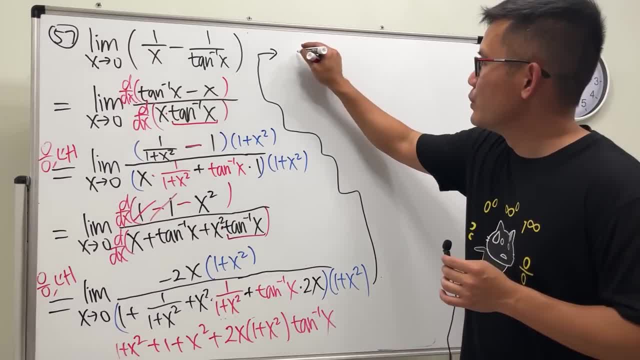 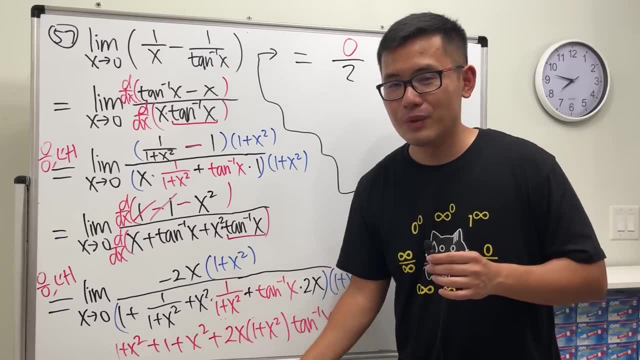 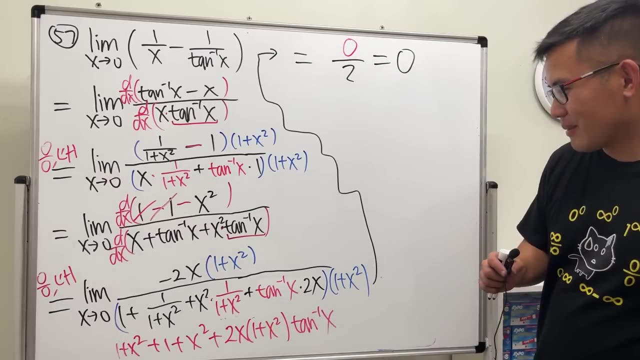 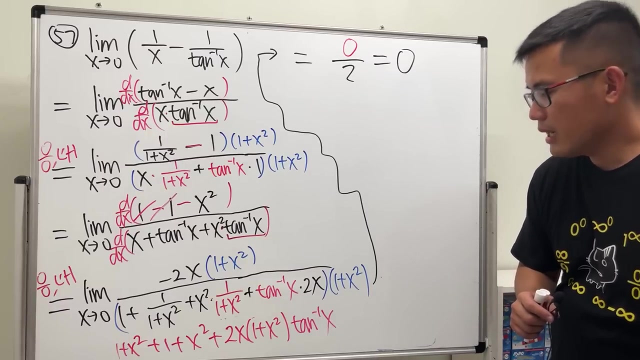 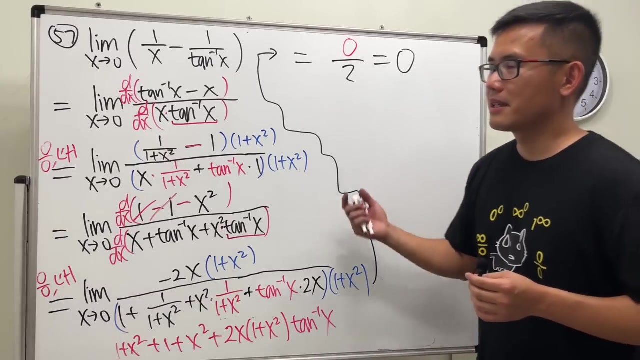 we get 0. so all in all, we just get 0 right, 0 over 2. what does that mean? the answer is just equal to 0. yes, need to double check. yeah, nothing wrong for sure. yes, to be right, 0, why not? huh, yeah, 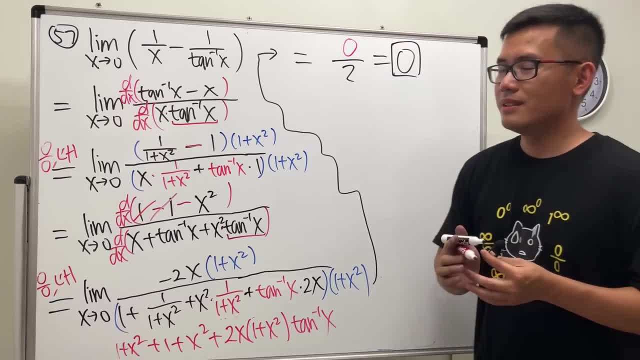 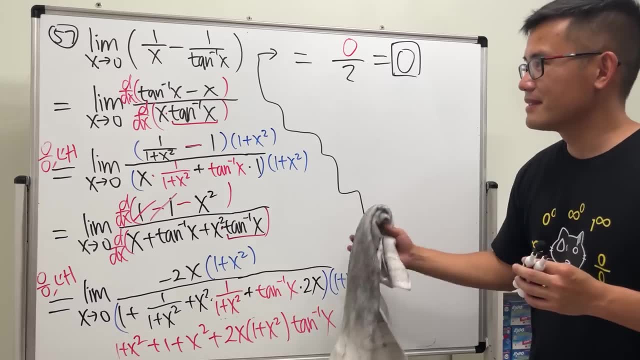 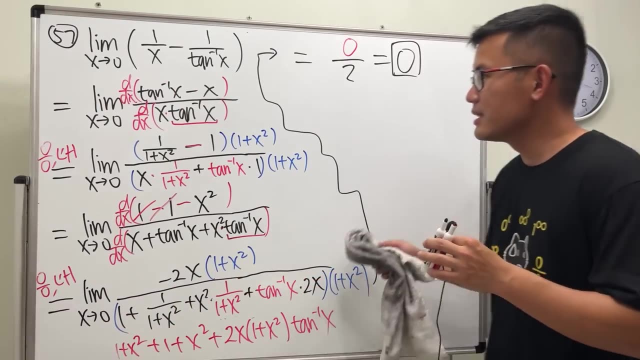 you guys can pause the video and just verify this with me, verify this for me and then just do it on your own, why not? it should be 0, right, alright, so 57 check good. 4 hours and 12 minutes. so far. so good, 57 is 0. 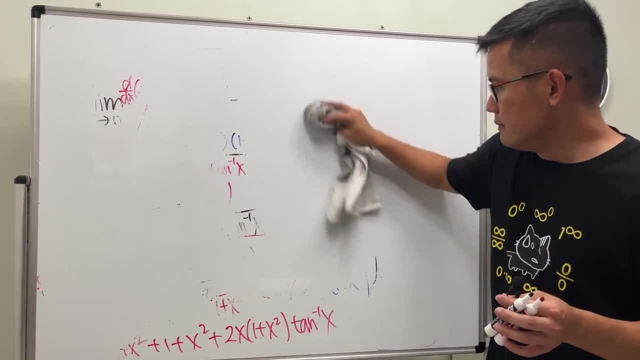 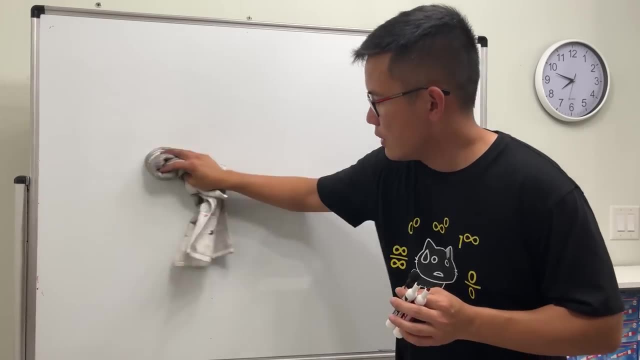 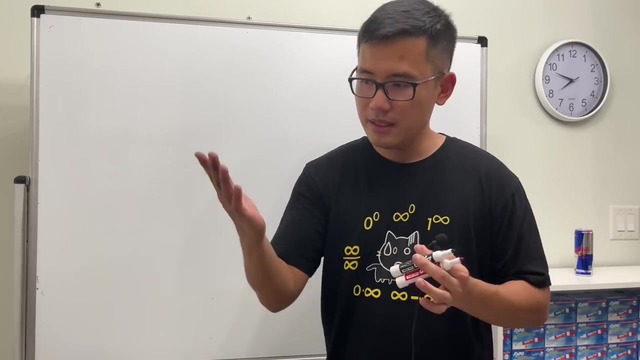 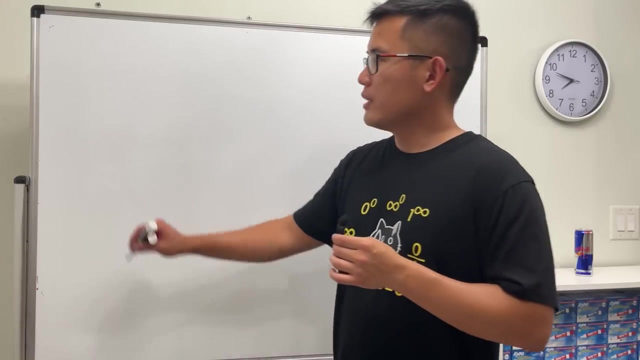 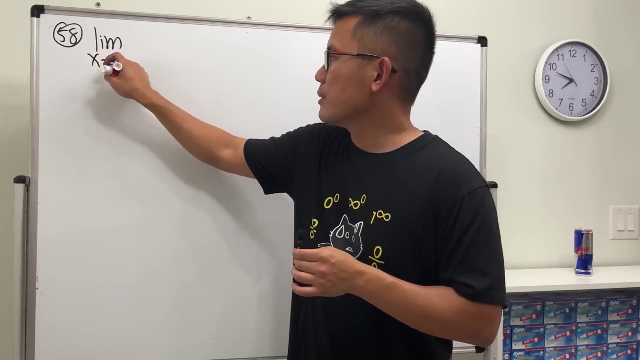 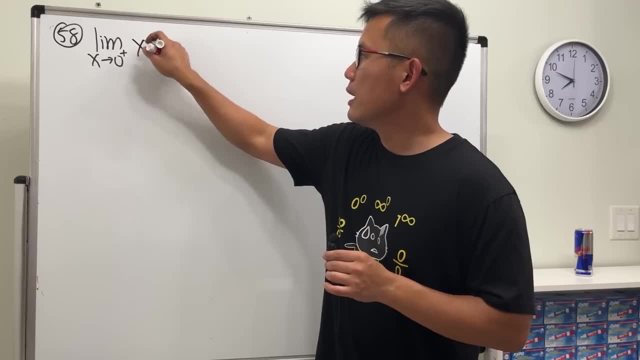 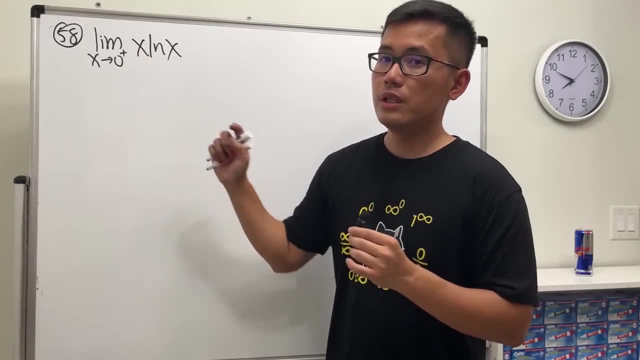 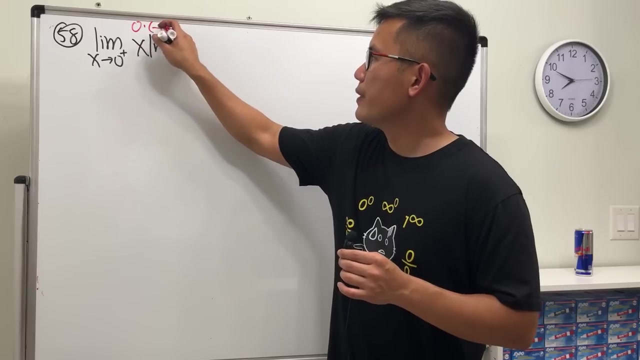 x times l and x, right? oh, ok, i can talk about another indeterminate form. check this out: when we put 0 into here, we get 0, and then when we put 0 plus into l and x, we get negative infinity, right? so yeah, it's like this. 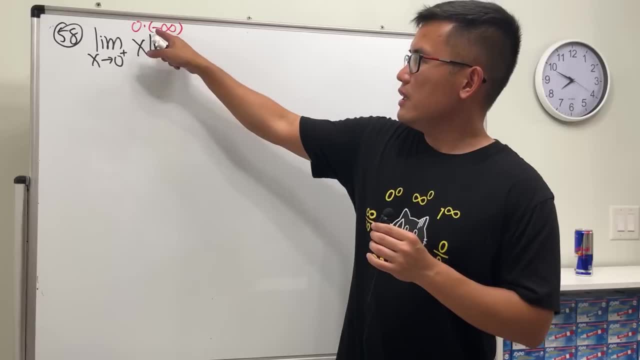 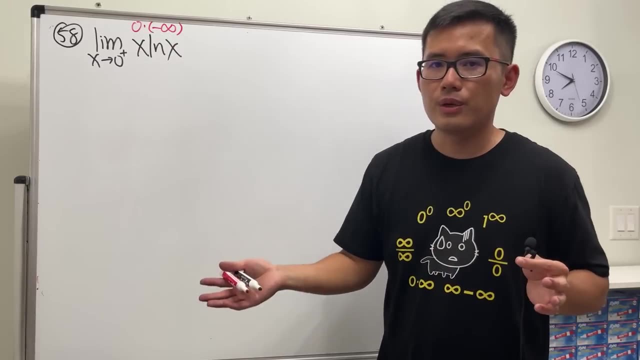 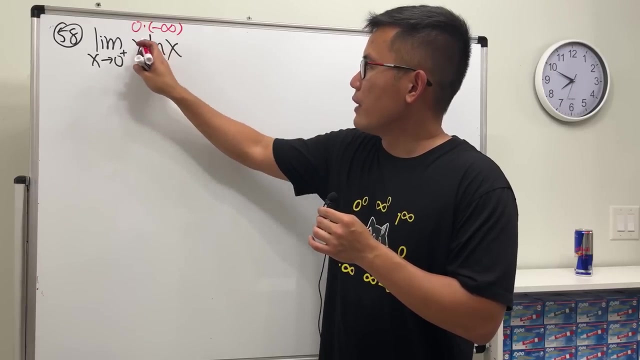 so we have 0 times infinity right here. the negative doesn't matter. we care about this times that, that indeterminate form, and that's no goal. we cannot draw any conclusion yet. why don't you stop it all through? how check this out? pick one of the functions. 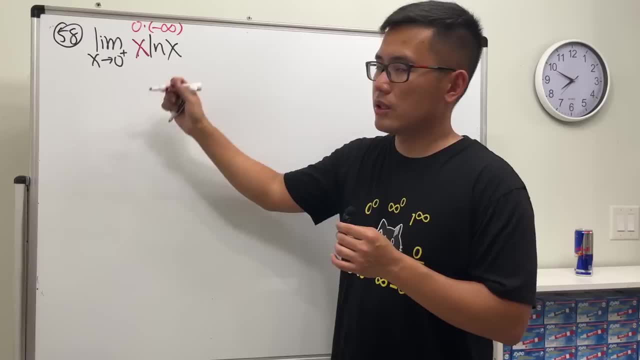 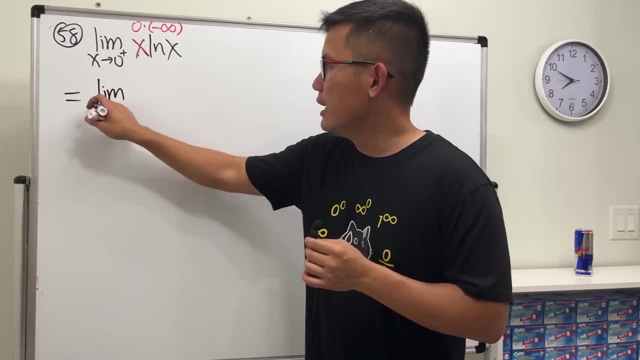 it will be easier if you pick x. just trust me on this, and then you want to bring this down down. i'll show you this right here. it's the same as the limit as x approaching 0, plus keep the l and x on the top, but then 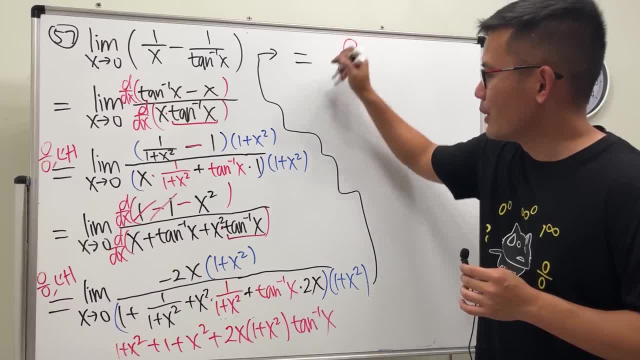 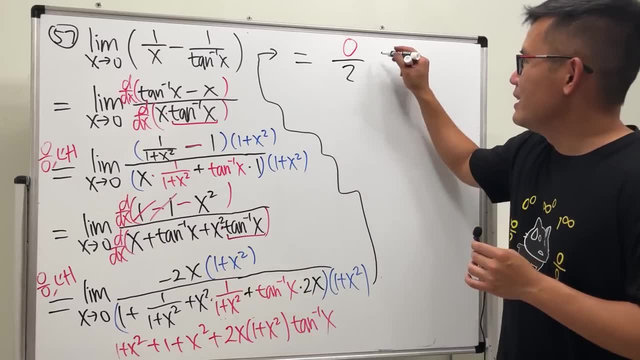 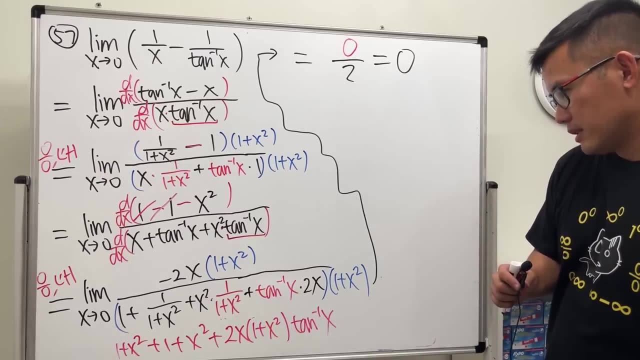 So all in all, we just get 0,. right, 0 over 2.. What does that mean? The answer is just equal to 0.. Oh Yes, Let's double check. Yeah, nothing wrong, For sure. 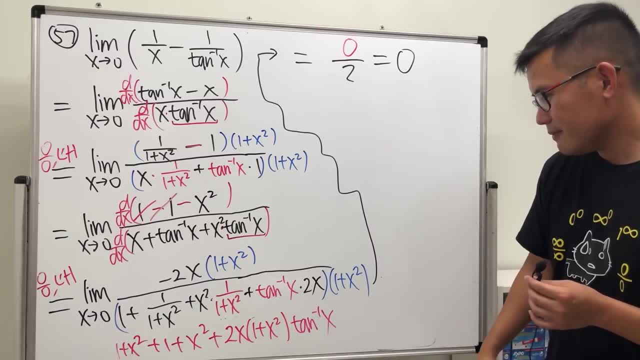 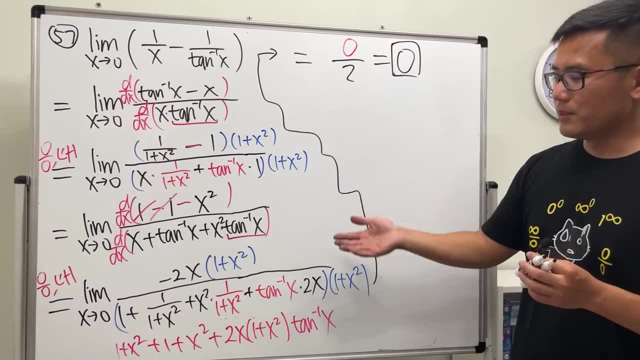 Yes to be right. 0, why not? huh Yeah, you guys can pause the video and just verify this with me. Verify this for me and then just do it on your own. Why not? It should be 0, right. 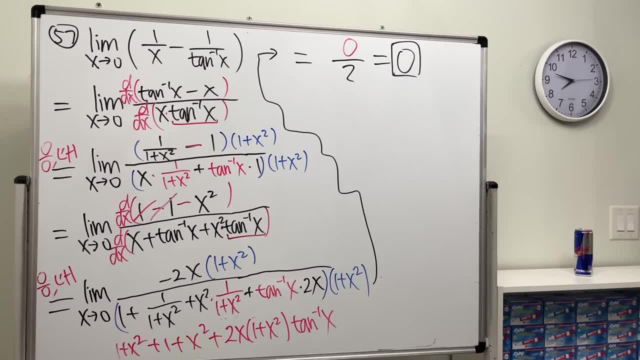 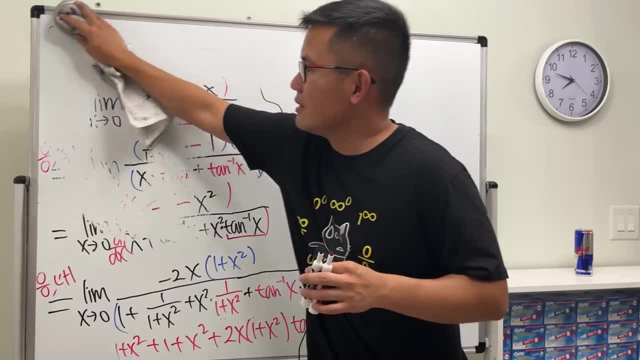 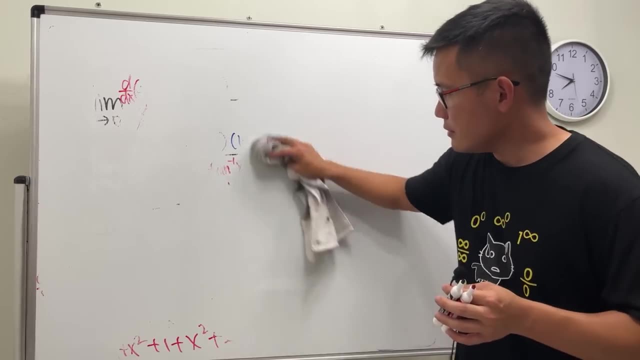 Alright, so 57, check good. 4 hours and 12 minutes. So far, so good. 57 is 0.. This is pretty good. Oh, what I was thinking? wait, you're gonna say 0 here, but there's always 0.. 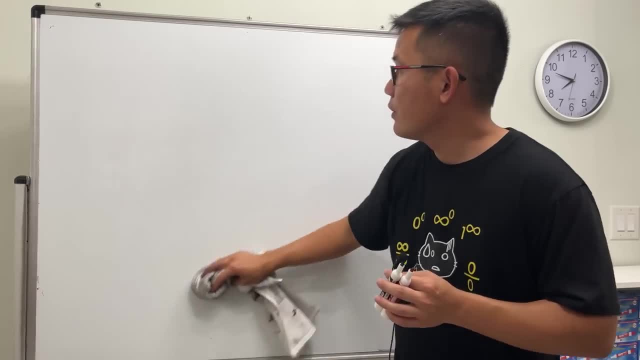 Yeah, And yeah, as I said, there's always 0.. And there's always 0.. A minute, there's always 0.. Yeah, yeah, there is always. So let's go over here. See, see, see, see. 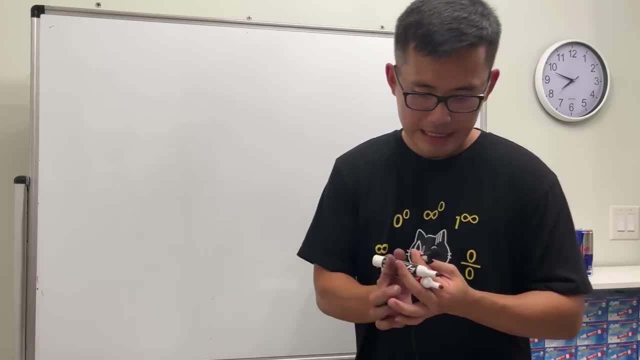 See, that's pretty easy. So we have 1, 2,, 3, 4,, 5, 6, 7, 6, 8,, 9,, 10,, 10, 10.. We're still here with 0.. 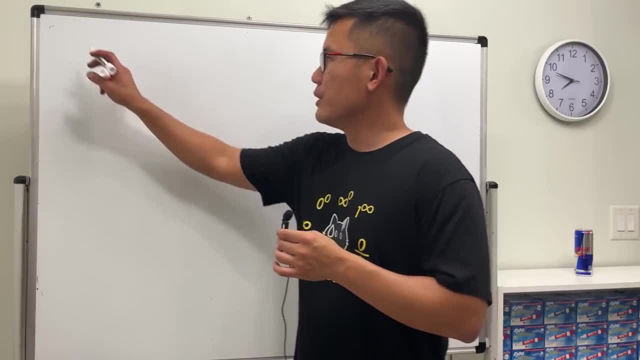 We're still here with 0.. So we can see the 0.. So here we are, we can see this: 1 here and a b 3, and a b 4, so we have 1.. And now we have, we have a b 3,. 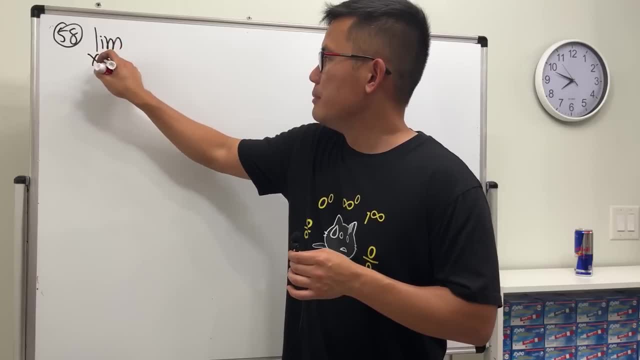 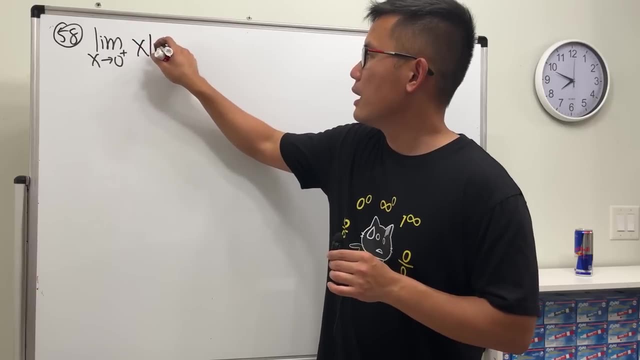 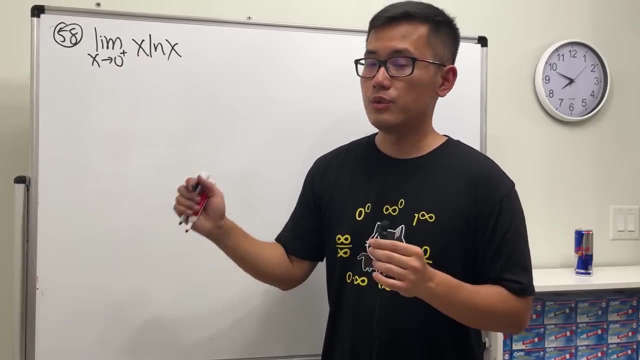 Gentle question: limit as x approaching 0 plus, and then we have x times ln x, right? Oh, okay, I can talk about another indeterminate form. Check this out: When we put 0 into here, we get 0, and then when we put 0 plus into ln x, we get negative infinity, right? 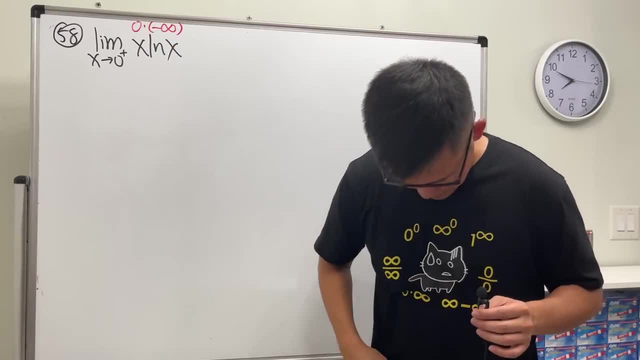 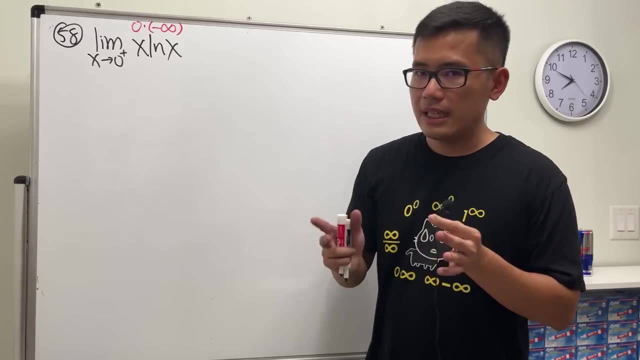 So yeah, it's like this. So we have a 0 times infinity right here. Okay, the negative doesn't matter, We care about this times, that indeterminate form, and that's no goal. We cannot draw any conclusion yet. 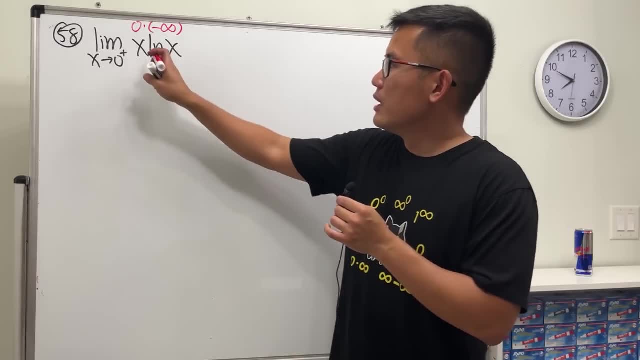 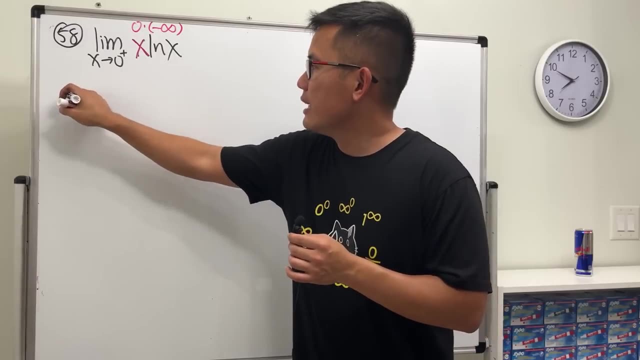 Why don't you use Doppler's rule? How Check this out? Pick one of the functions. It will be easier if you pick x. Just trust me on this, And then you want to bring this down down, I'll show you. 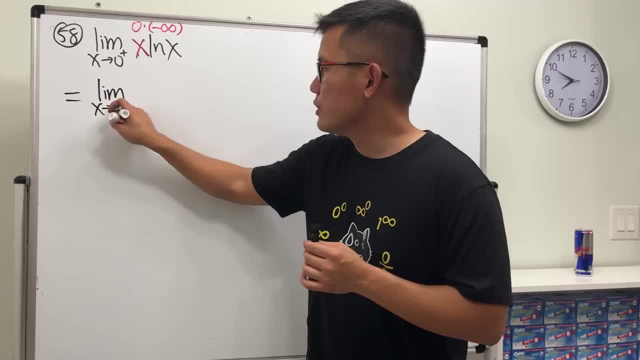 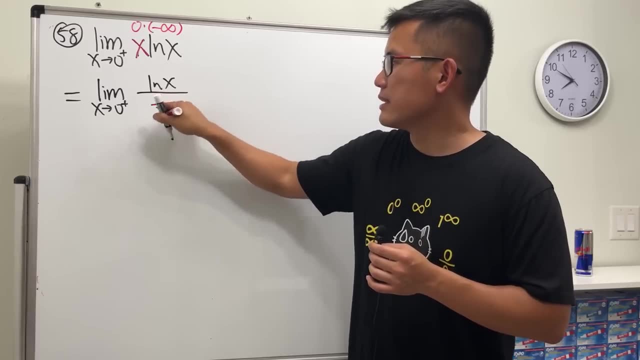 This right here is the same as the limit as x approaching 0, plus Keep the ln x- It's on the top- but then change the x to 1 over x on the denominator, because now you can see, if you multiply the top and bottom by x, then you get the original back. 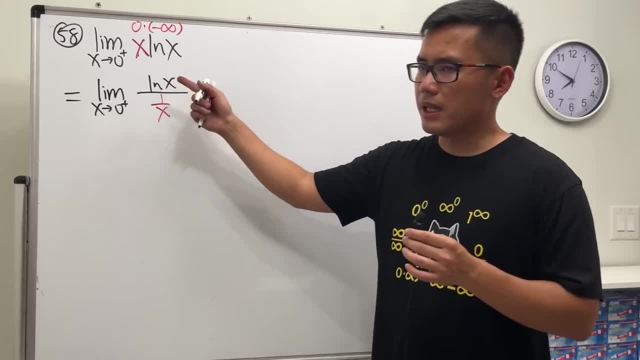 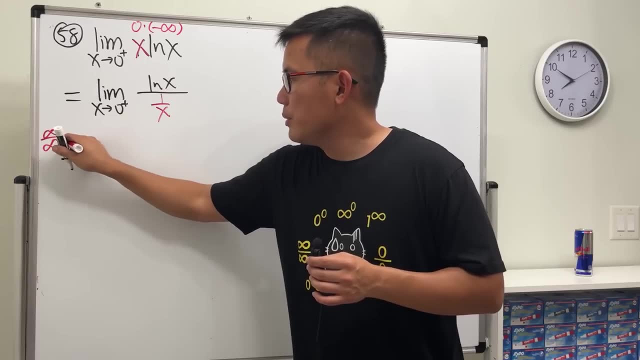 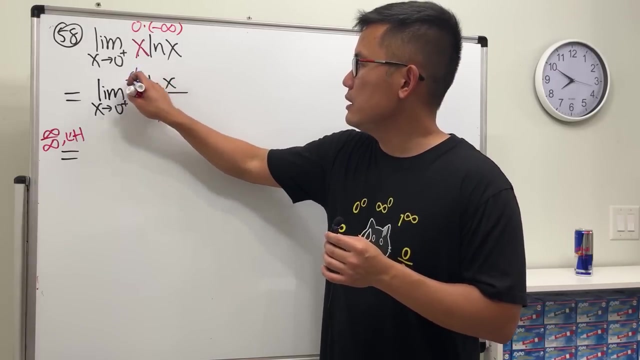 Cool huh. Now if you put 0 or 0 plus in here and here, you get infinity over infinity. So we are able, we can actually allow, we are allowed to use Lapito's rule now. So I will put this down: d dx. 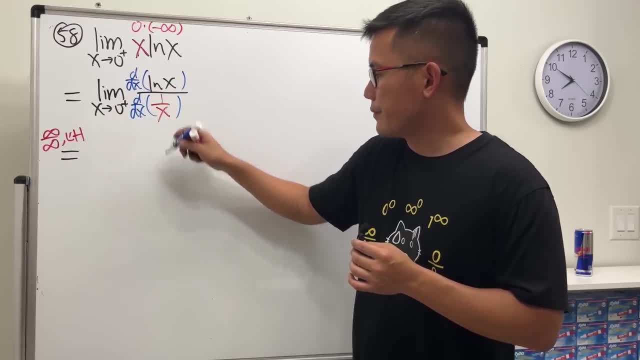 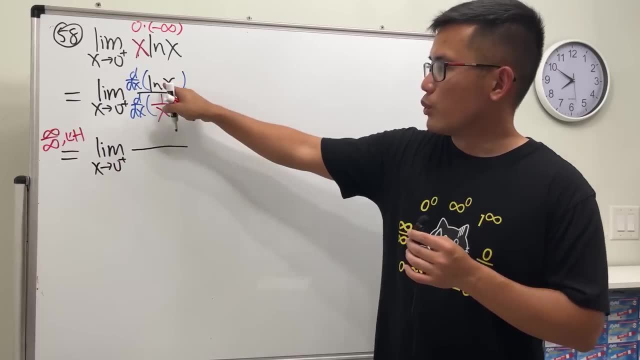 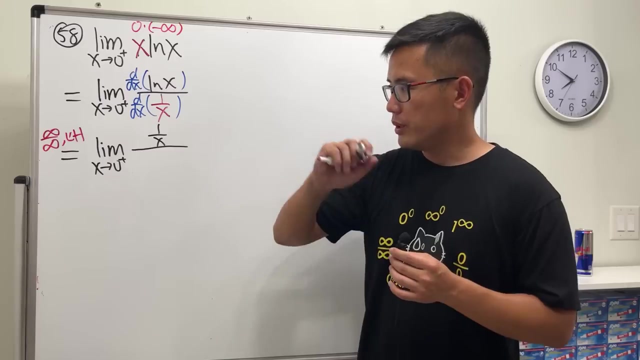 All right. So here we have the limit as x approaching 0 plus. The derivative of this is 1 over x. The derivative of this rightly as x to the negative 1 power, bring the negative 1 to the front minus 1.. 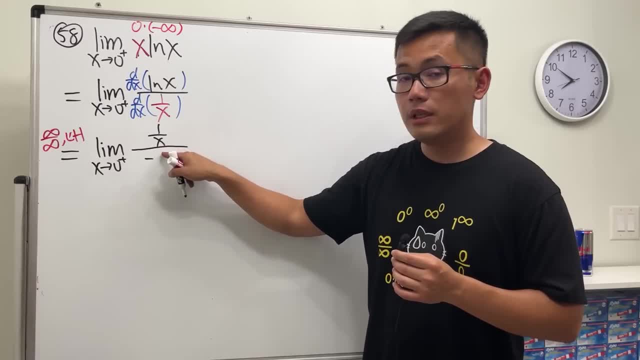 So it's negative x to the negative 2 power, which is just negative 1 over x squared. Before we plug in the derivative of x to the negative 1 power, we are able to find the derivative of x to the negative 1 power. 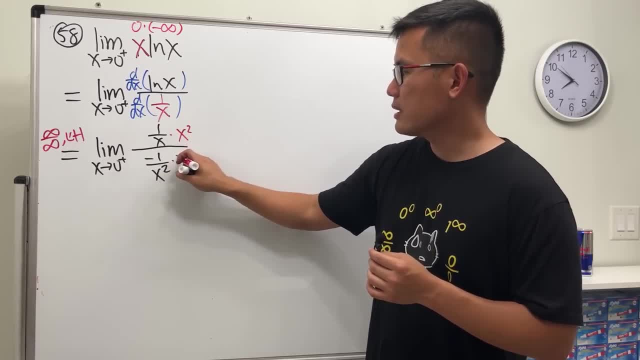 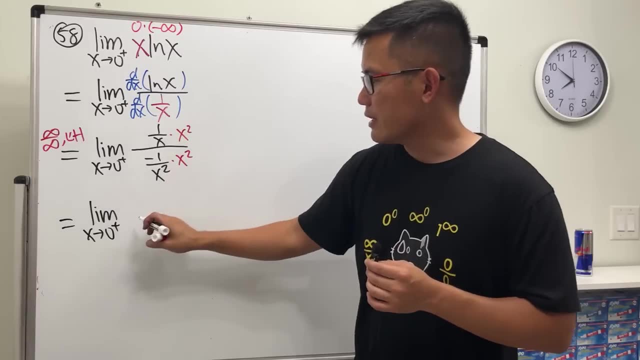 Before we plug in 0, let's just simplify it. Multiply the top and bottom by x squared, And then we will see. this is the limit. as x approaching 0 plus We have a negative, They cancel And then they reduce to just x. 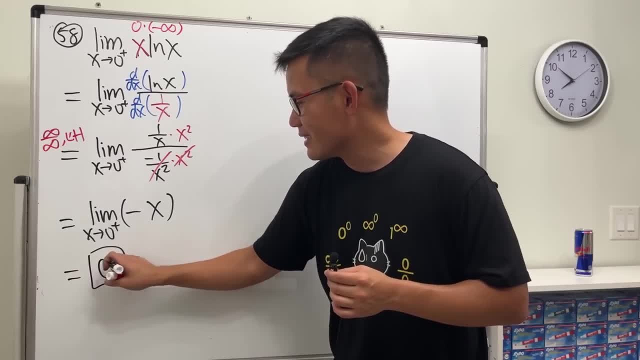 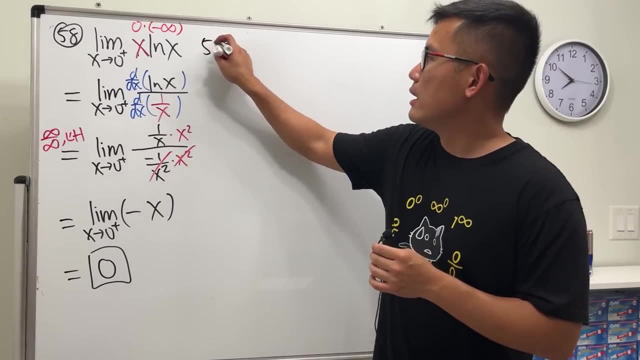 Put 0 in here we get 0.. Yes, Oh, my goodness, Another 0.. Not so satisfying, but that's just how it is Okay. Okay, Please Do not say 0.. 0 times infinity or 0 times negative infinity is equal to 0 all the time. 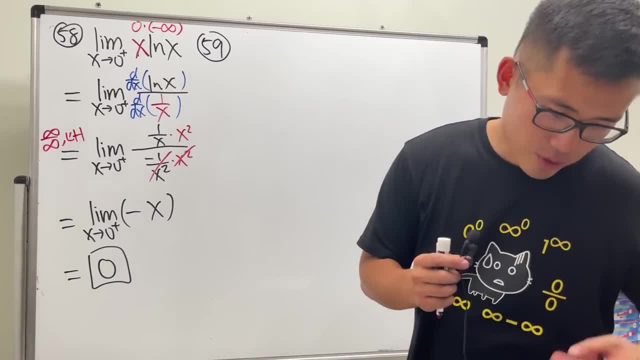 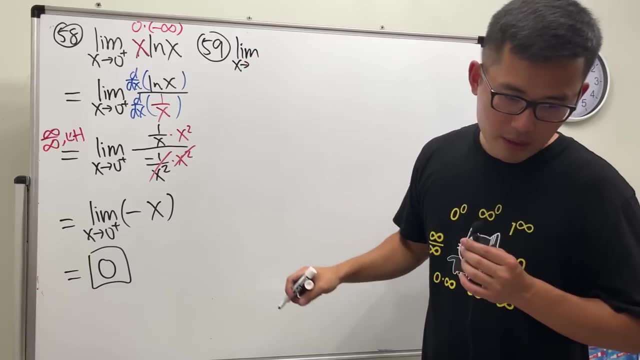 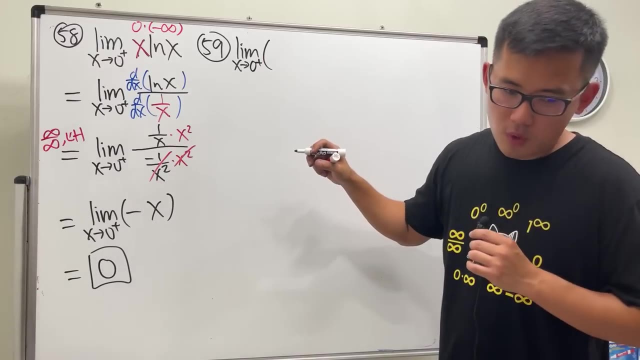 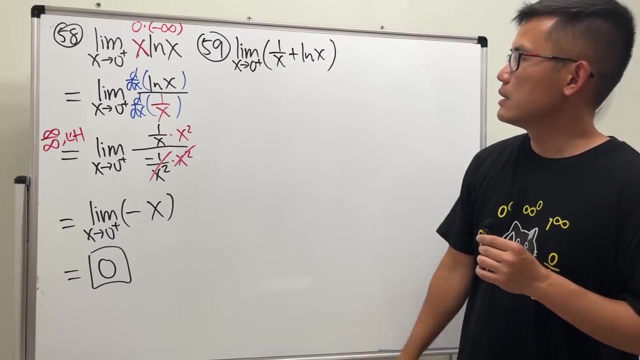 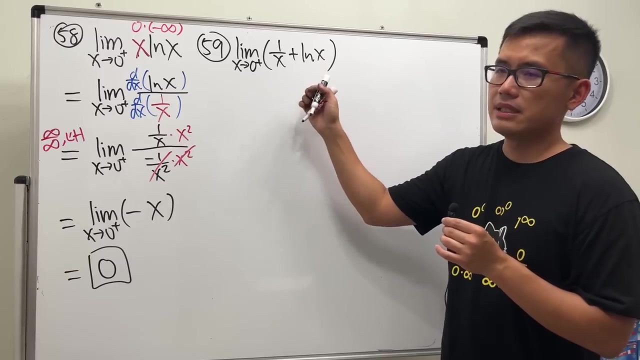 Sometimes it is, but not all the time. Okay, Let's try another one, Number 59. Limit as x approaching another 0 plus 1 over x plus ln x. Now here's the deal: If you put 0 plus in here and here, you get infinity and then minus infinity. 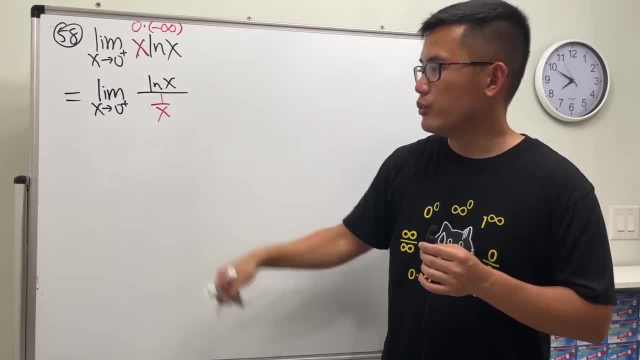 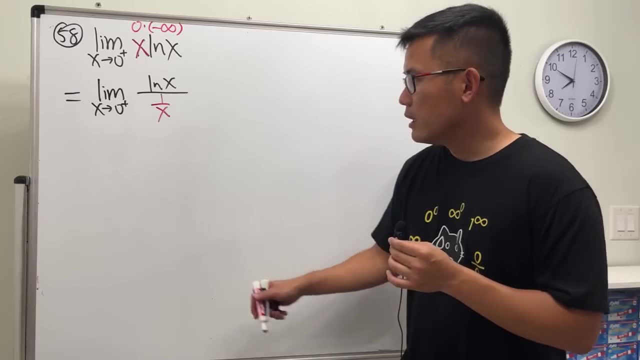 change the x to 1 over x on the new, on the denominator, because now you can see, if you multiply the top and bottom by x, then you get the original back. cool huh. now if you put 0 or 0 plus in here and here, you get infinity over infinity. 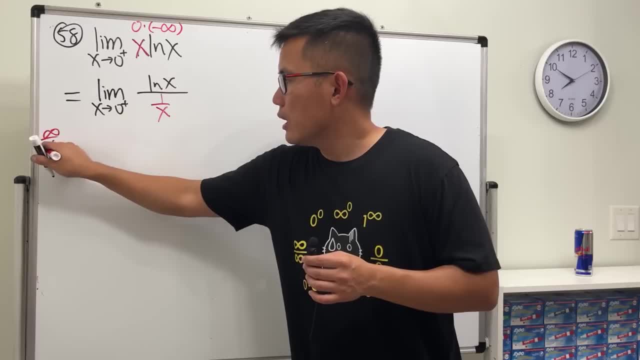 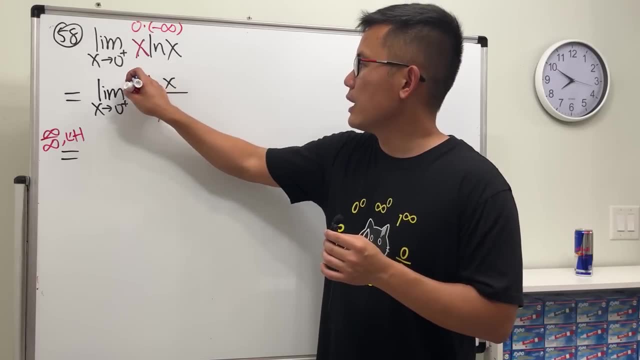 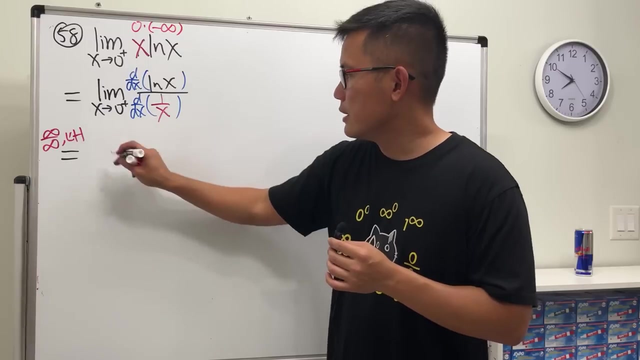 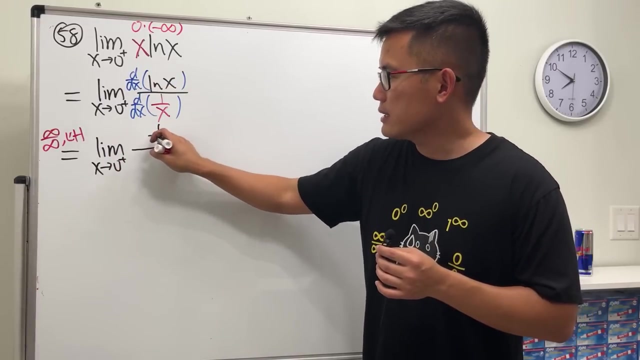 so we are able, we can actually allow, we are allowed to use lapito's rule now. so i will put this down: d, dx, d, dx, and alright. so here we have the limit as x approaching 0, plus the velocity of this is 1 over x. the. 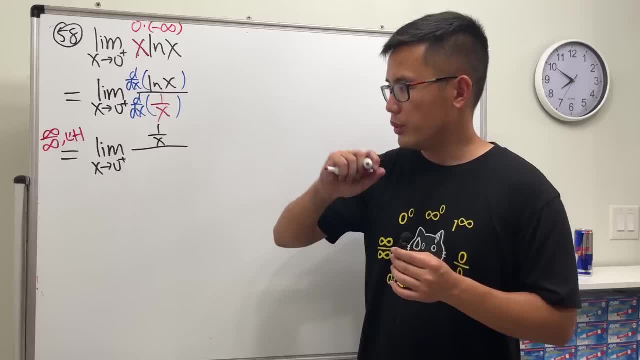 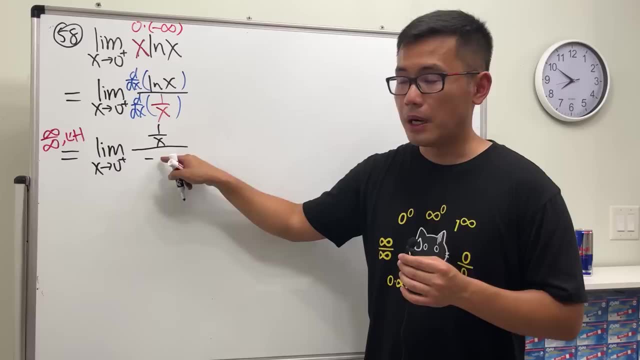 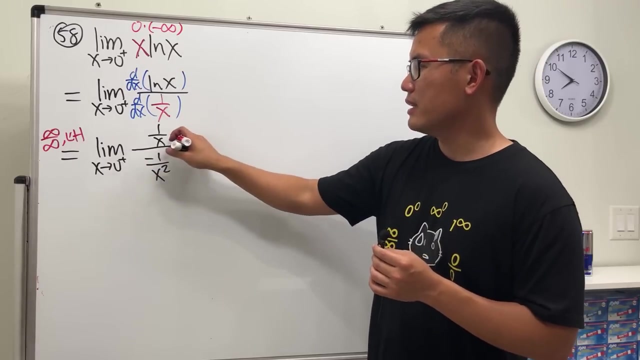 velocity of this rightly as x to the negative one power. bring the negative one to the front minus one, so it's negative x to the negative two power, which is just negative one over x square. before we plug in 0, let's just simplify it. multiply the top and bottom by x. 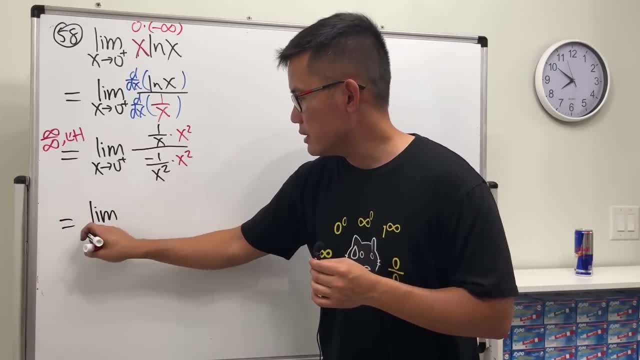 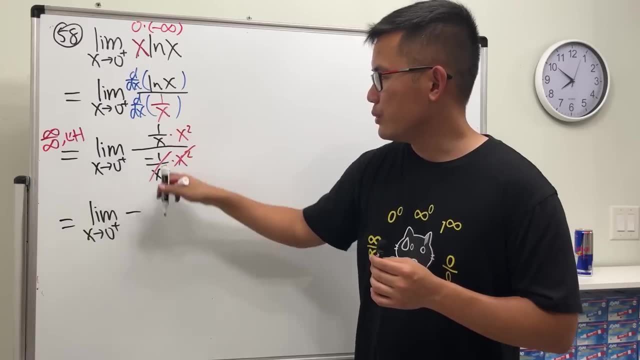 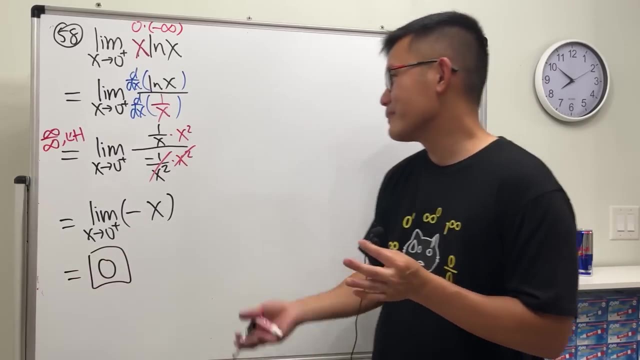 and then we will see: this is the limit. as X approaching 0 plus we have a negative, they cancel and then they reduce to just X. put 0 in here, we get 0. yes, oh, my goodness, another 0. not so satisfying, but that's just how it is. 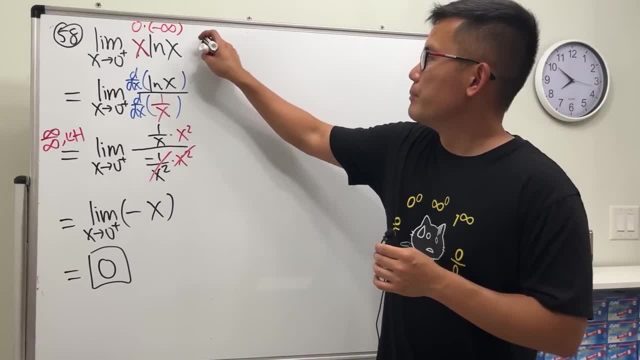 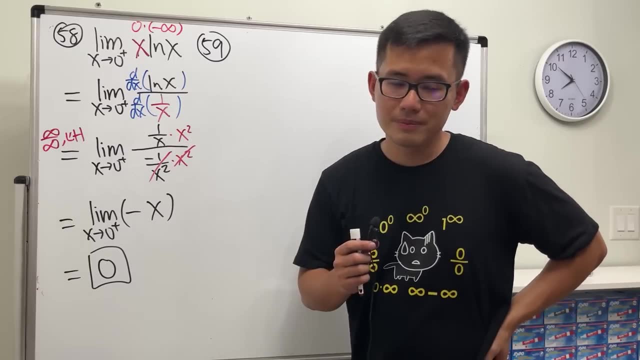 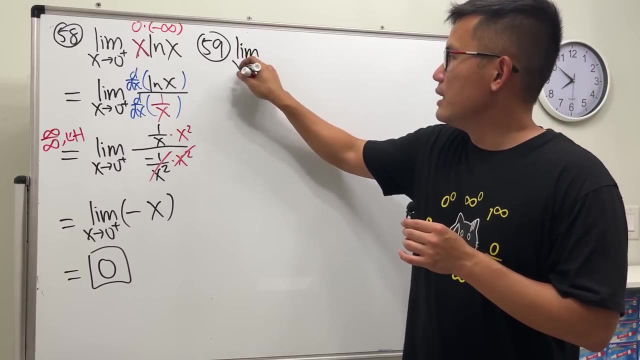 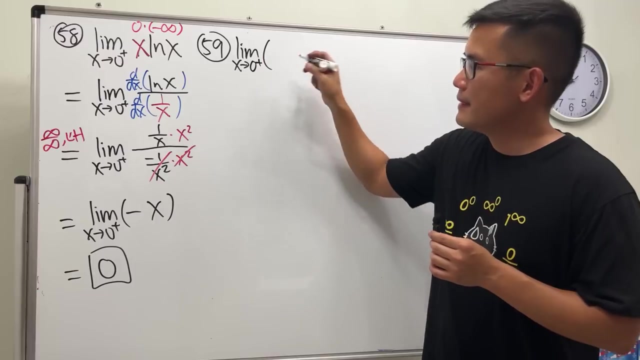 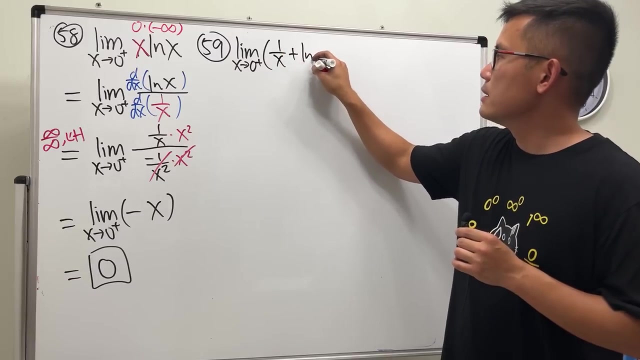 okay, please do not say 0 times infinity or 0 times negative. infinity is equal to 0 all the time? sometimes it is, but not all the time. okay, let's try another one number: 59 limit as X approaching another 0 plus 1 over X plus L N X. now here's the. 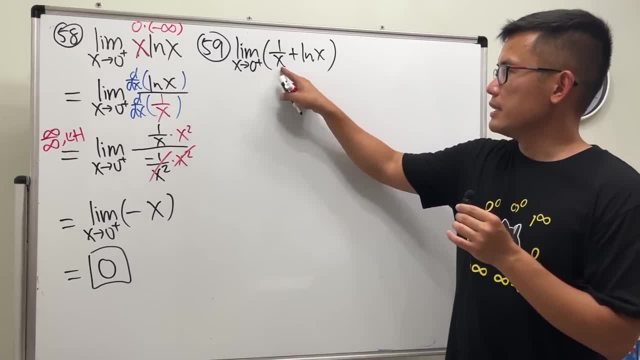 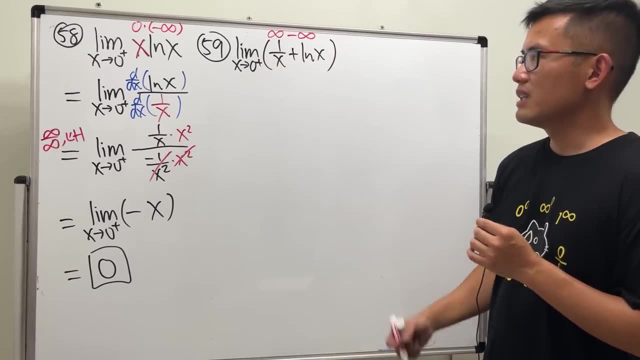 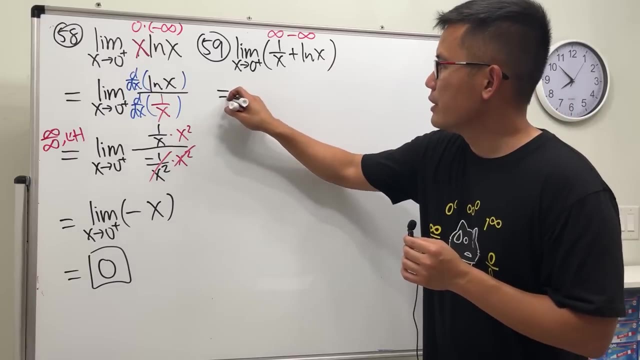 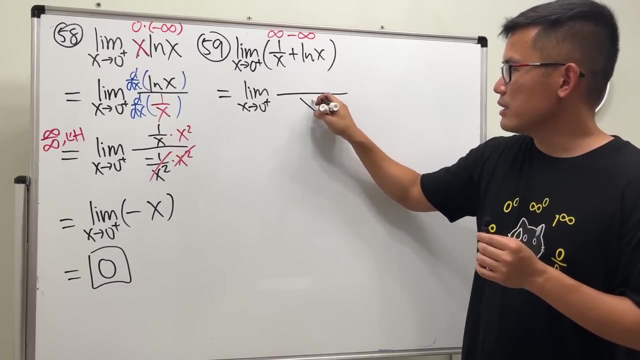 deal if you put 0 plus in here and here you get infinity and then minus infinity. so this is the infinity minus infinity situation. again, let's just combine the fractions and let's see how this goes. huh, so this right here equals the limit as X approaching 0 plus multiply X and X. right, so we just have X here and then we. 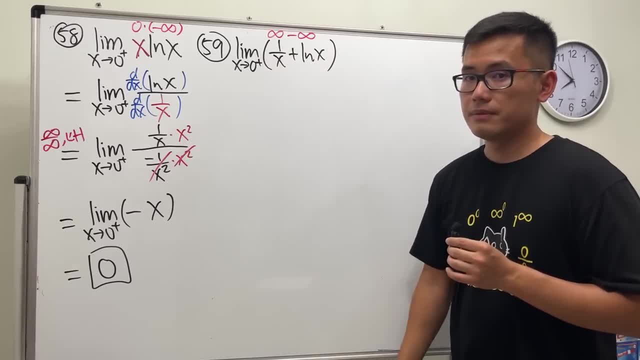 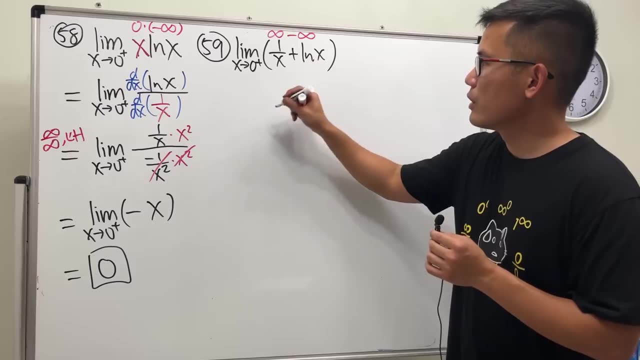 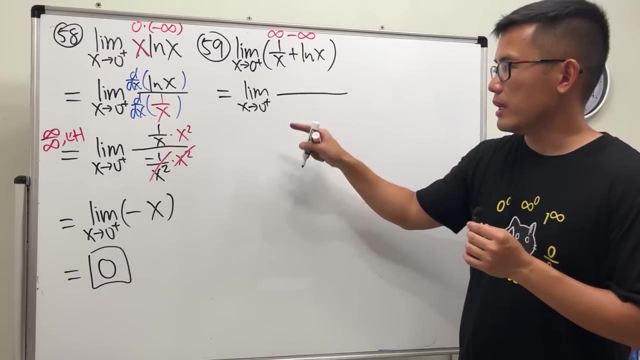 So this is the infinity minus infinity situation. Again, let's just combine the fractions and let's see how this goes. So this right here equals the limit as x approaching 0 plus Multiply x and x, right, So we just have x here and then we have 1 plus and we get x times ln x. 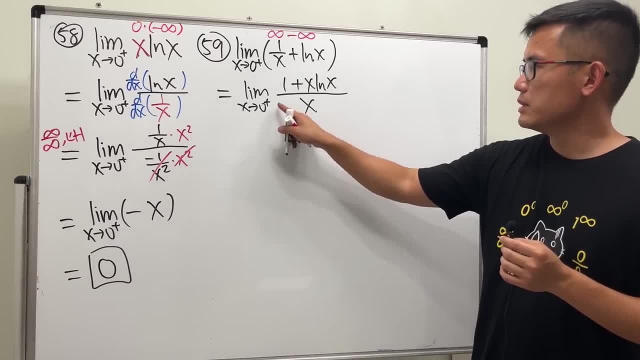 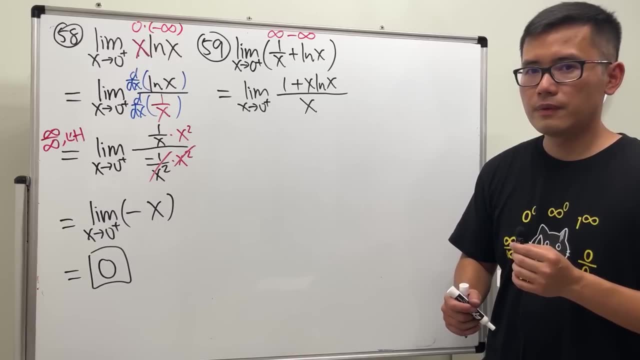 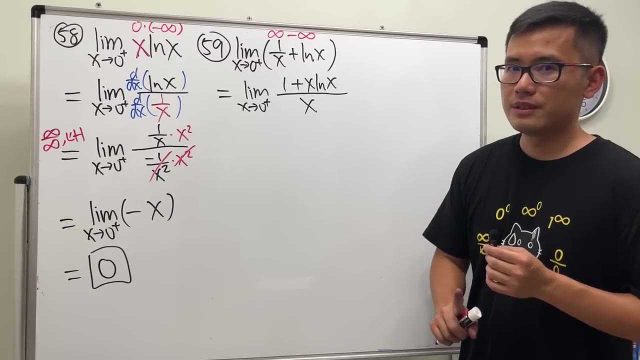 But check this out: If we put 0 plus into all the x's, what do we get? Should we just do Lapito's rule right now? Can we just do Lapito's rule and say, no, do not do Lapito's rule right now. 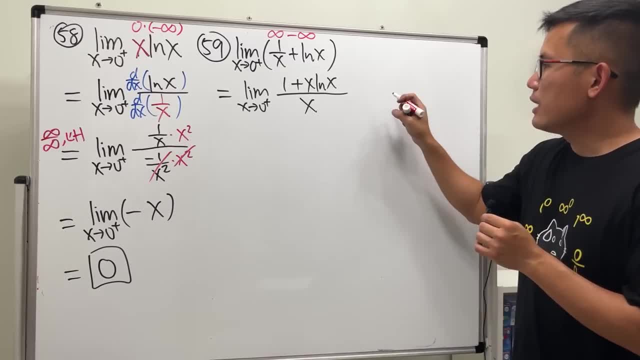 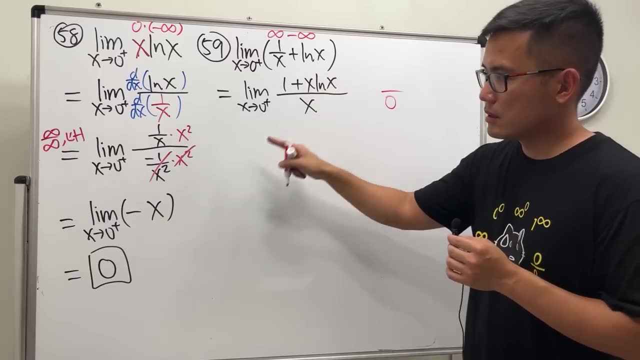 Why? Why? Because if you put 0 plus in here, on the bottom we get 0.. On the top, hey, what's x? Times ln x. We did it earlier and then it's the same thing, But we have a 1.. 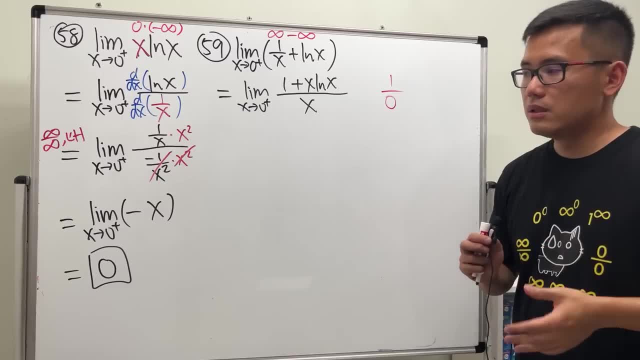 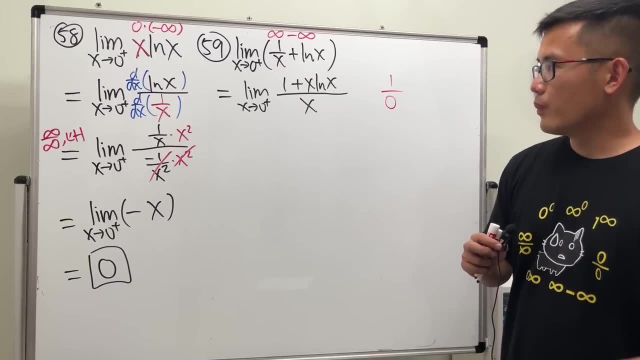 So, in fact, we end up with 1 over 0. This is 1 over 0.. So what do we do next? Well, you don't have to worry about doing Lapito's rule in this case. We kind of did it for this part, right here. 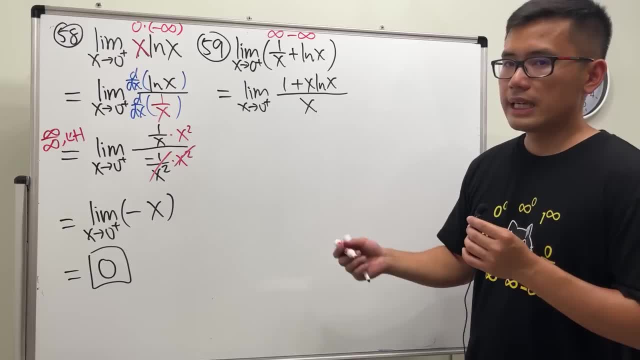 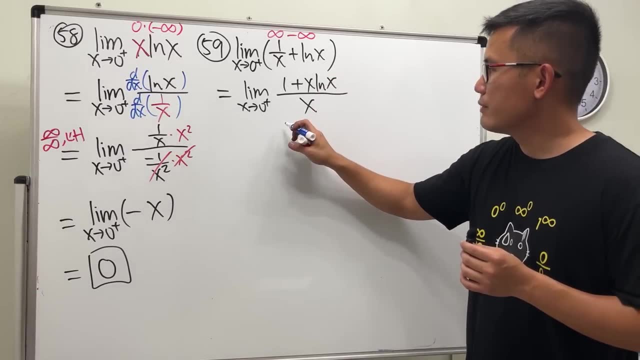 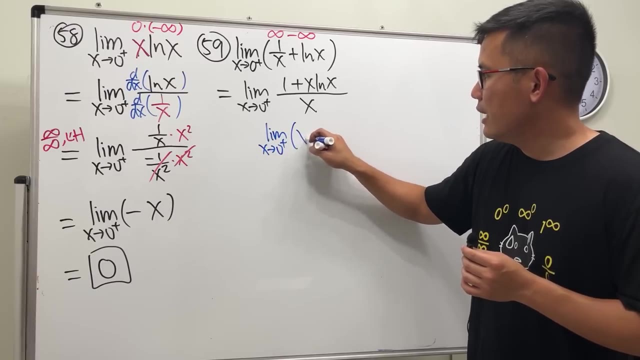 But the truth is. the truth is we can actually kind of argue what the answer should be already, So I will just have to say this part: the limit as x approaching 0 plus x, ln, x, This right here is equal to 0.. 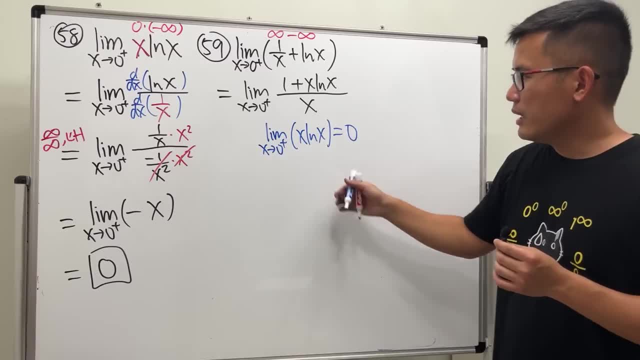 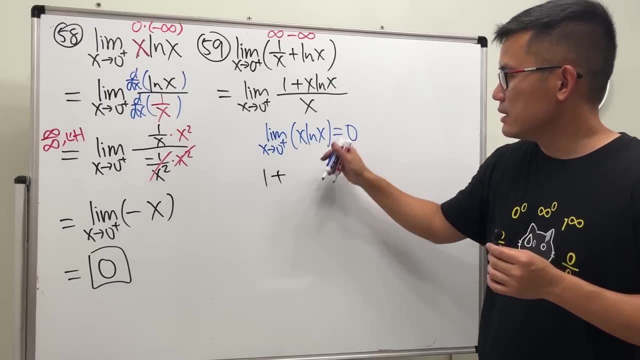 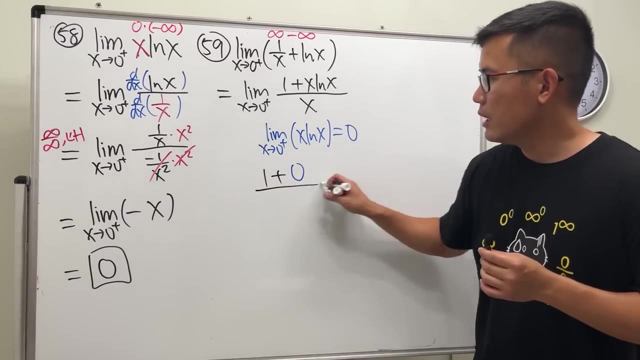 We did that for 58. So I can say that We can use it, And then you can see, this is just going to be 1 plus, this is 0. Because what we did earlier, And then we have x, is approaching 0 plus. 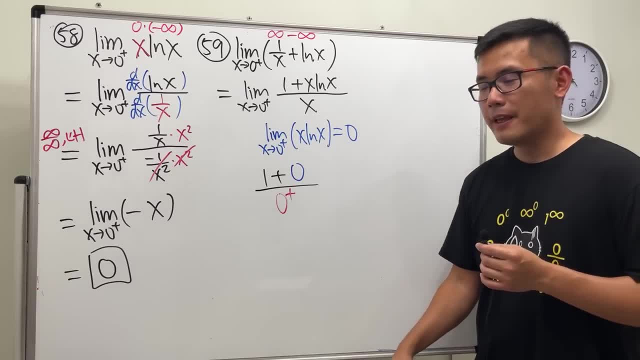 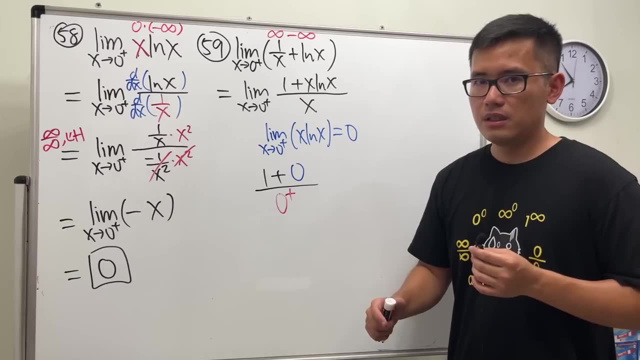 So the bottom here is 0 plus, And you might be wondering that is this 0 plus or 0 minus, Doesn't matter, because we're adding 1.. So the top is, for sure, positive. For sure it's a positive, non-zero number and divided by 0 plus. 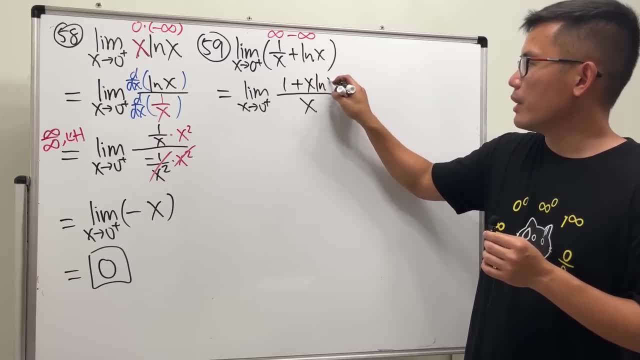 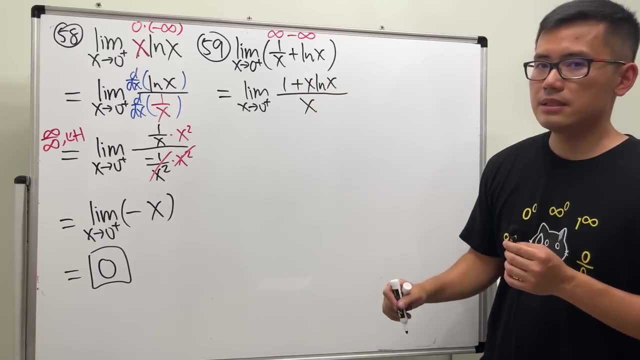 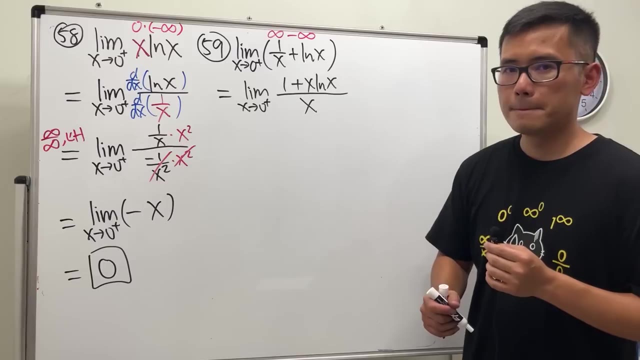 have 1 plus and we get X times L and X. but check this out: if we put 0 plus into all the X's, what do we get? so we just do Lapito's rule right now can we just do Lapito's rule and say: 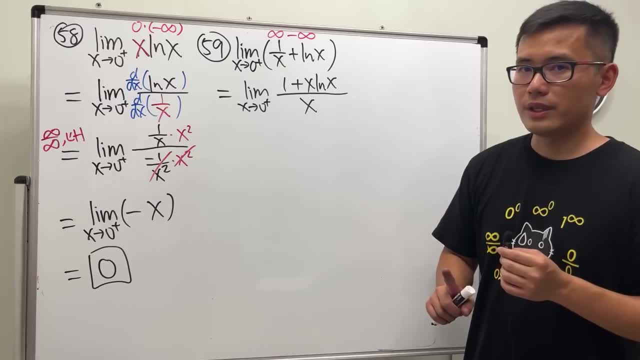 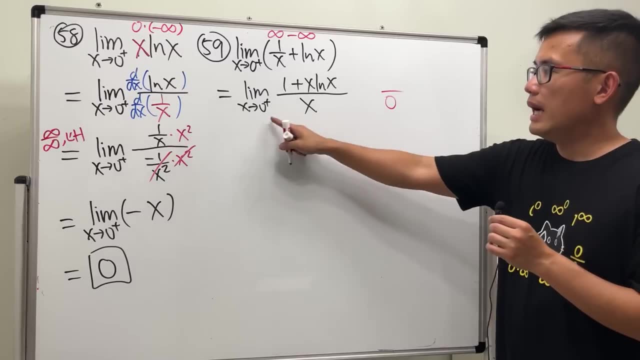 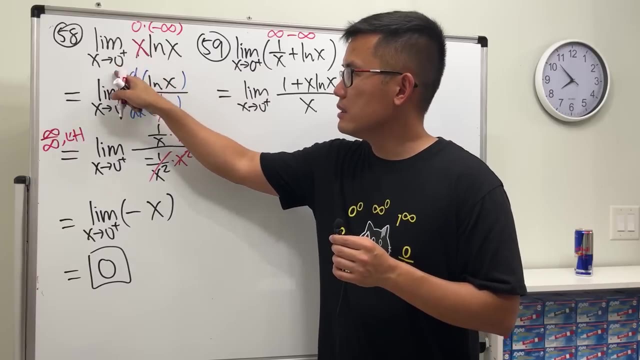 no, don't not do Lapito's rule right now. why? because if you put 0 plus in here on the bottom, we get 0 on the top. hey, what's X times L and X? we did it earlier and then it's the same thing, but we have a 1, so in fact we end up with 1 over 0. 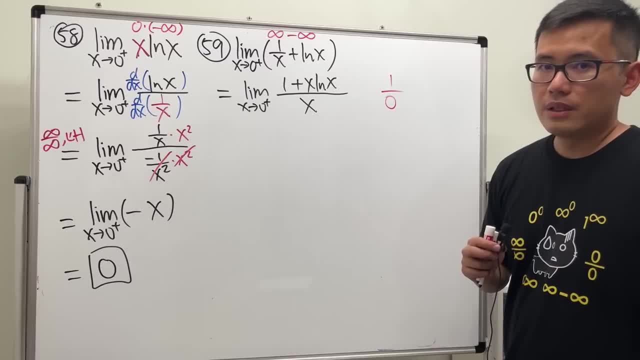 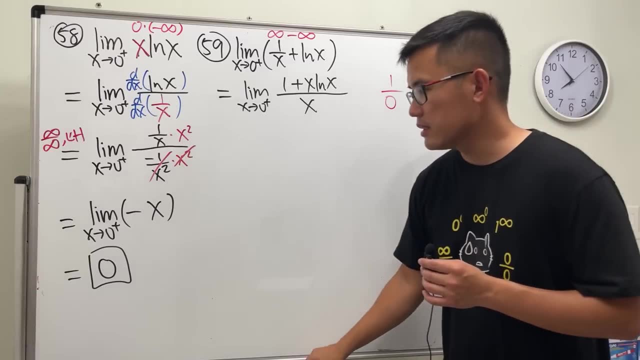 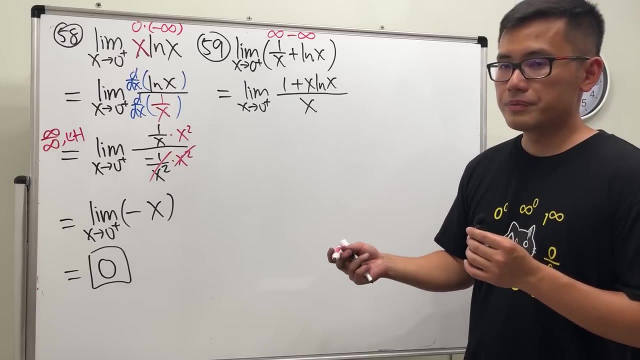 this is 1 over 0. so what do we do next? well, you don't have to worry about doing Lobito's ring this case. we kind of did over this part right here. but the truth is, the truth is we can actually kind of argue what the answer should be already. 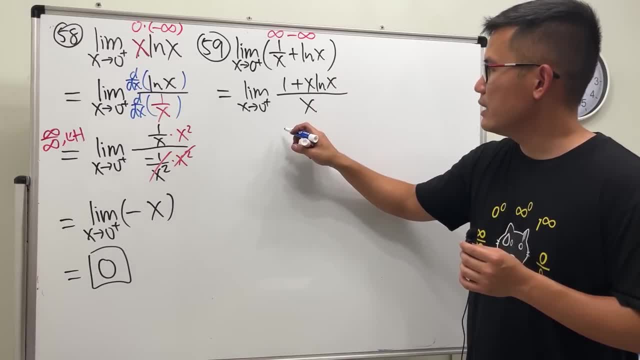 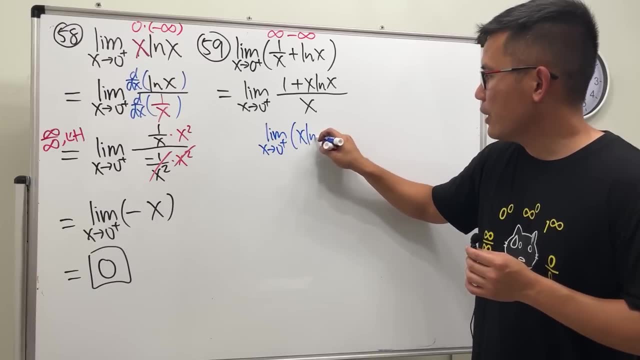 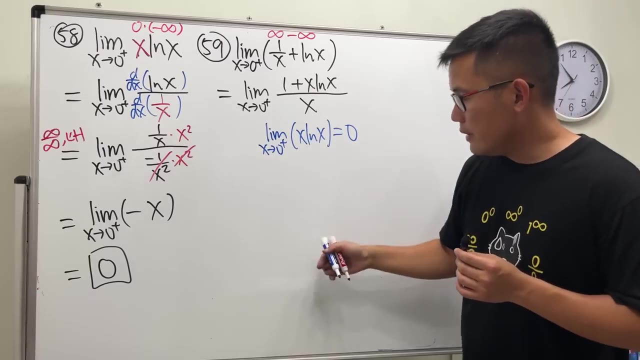 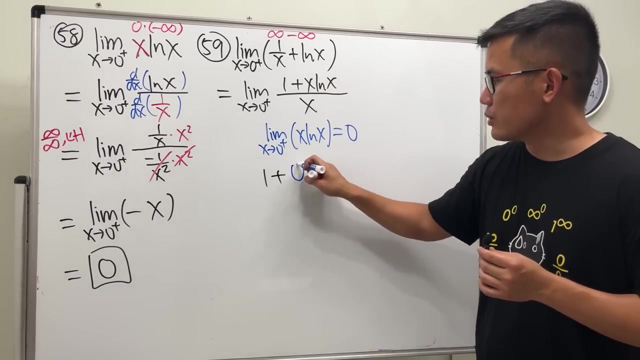 so I will just have to say this part. the limit as X approaching 0 plus X, L and X, this right here is equal to 0. we did that for 58, so I can say that we can use it and you can see this is just going to be 1 plus. this is 0 right because for 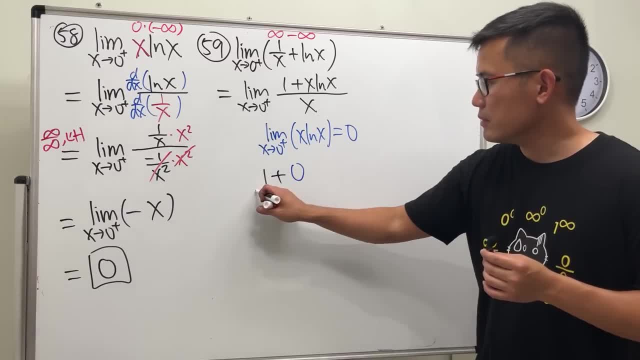 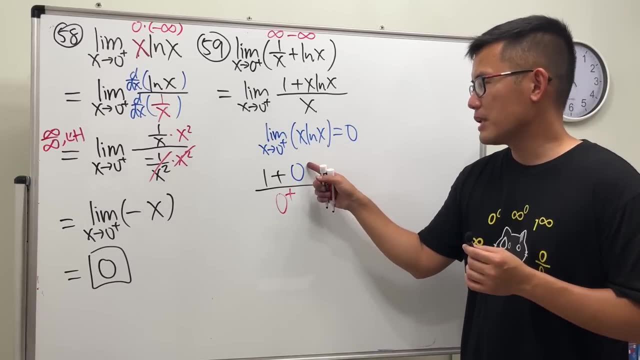 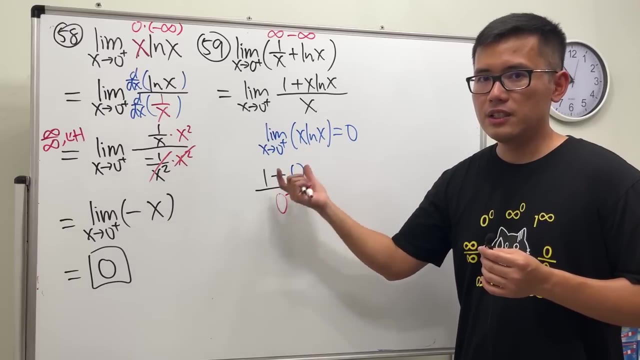 with the earlier. and then we have X is approaching 0 plus. so the bottom here is 0 plus, and you might be one day nice. this 0 plus was 0 minus, doesn't matter, because we're at 1. so the top is for sure positive. for sure it's a positive, a non-zero number and divided. 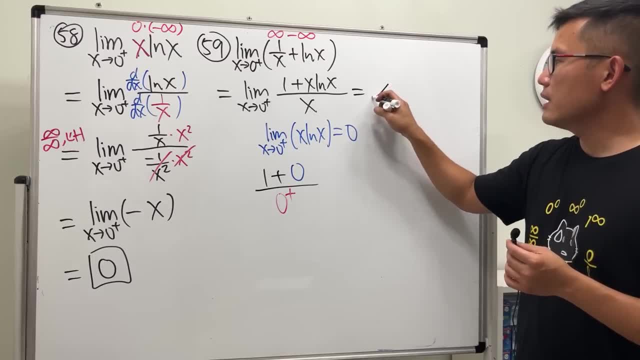 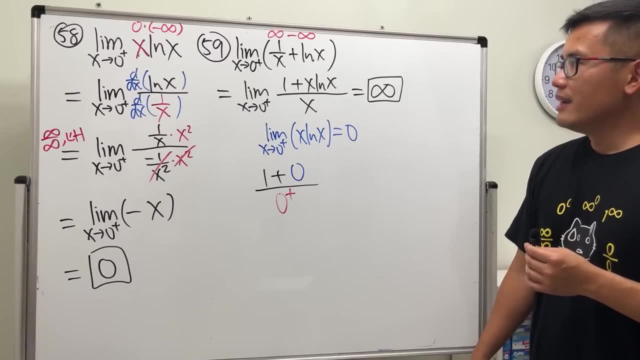 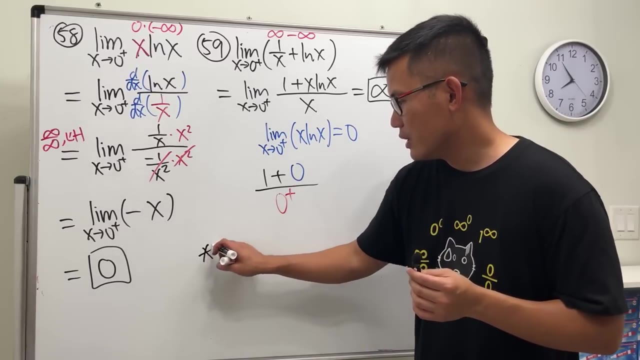 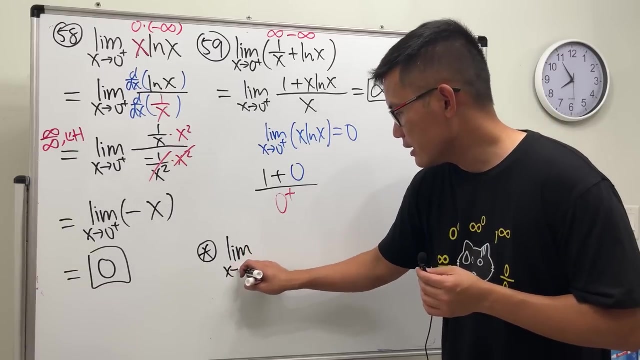 by 3 plus. so the answer for this is: what positive infinity? that's it, yeah. that's it, yeah. if you don't think this is like 100% legit, then you can also do it this way: you can factor out the 1 over X. this, right here, is the limit as X approaching. 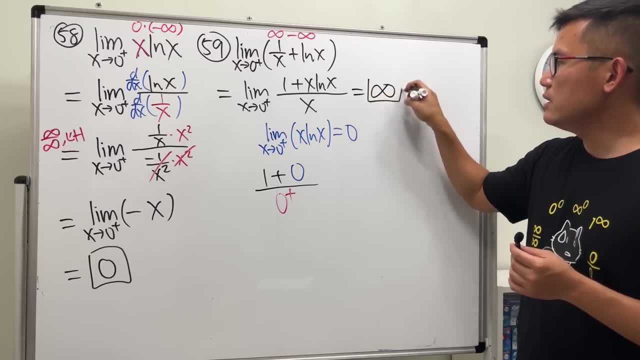 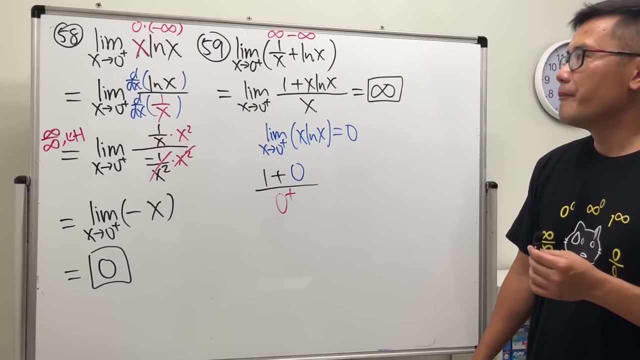 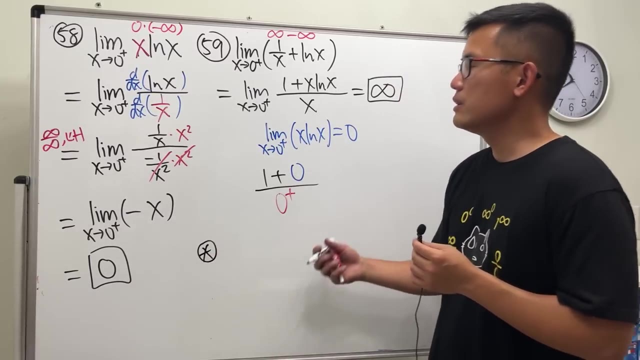 So the answer for this is: what Positive infinity. That's it, Yeah, that's it, Yeah. If you don't think this is like 100% legit, then you can also do it this way: You can factor out the 1 over x. 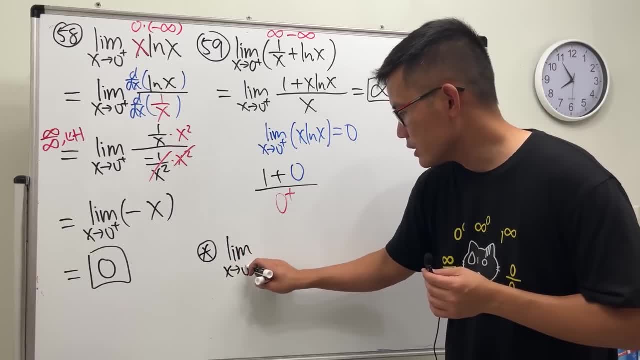 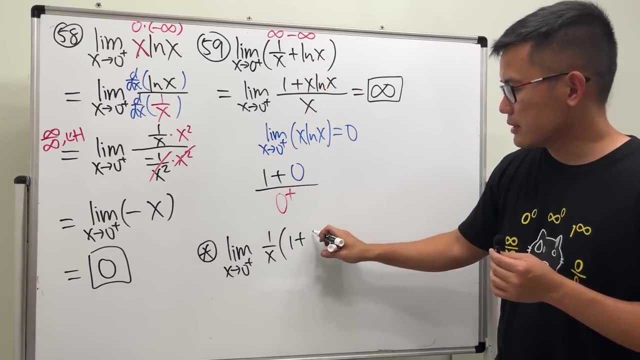 This right here is the limit as x approaching 0 plus, And then factor out the 1 over x And then you will get 1 plus. If you factor out 1 over x, it's like x times ln, x, Right. 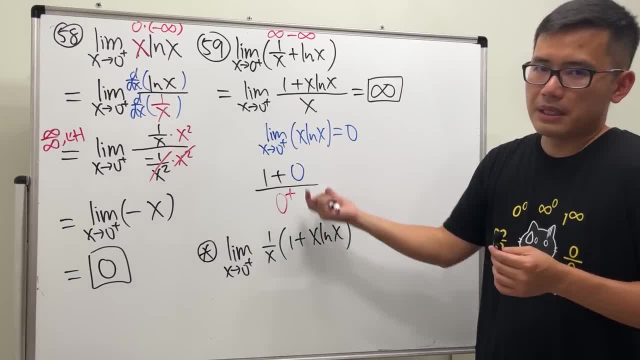 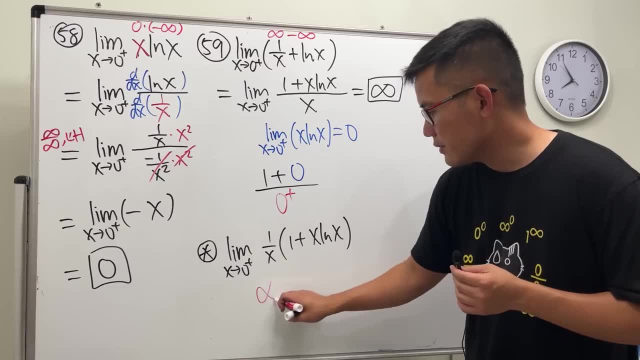 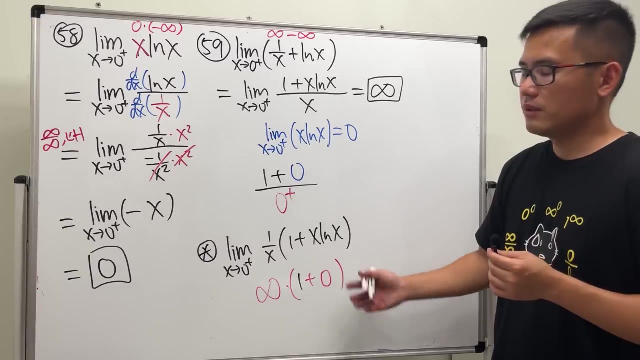 And it's pretty much like this, but like another look And you will see If you put 0 plus in here, this part is positive infinity, But this is 0. It's just like 1 plus 0. So infinity times 1 is infinity. 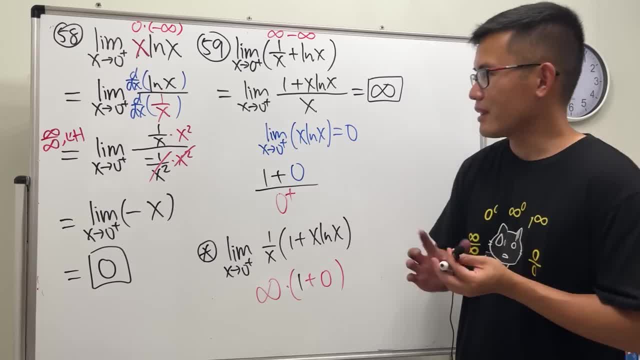 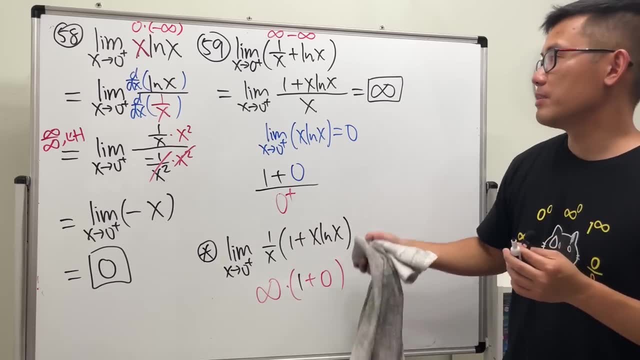 Yeah, So another way to look at it, But thanks to this part. Imagine if this right here turns out to be negative: 1. Then this question will be harder, but it's not. And you see, infinity minus infinity gives us infinity. 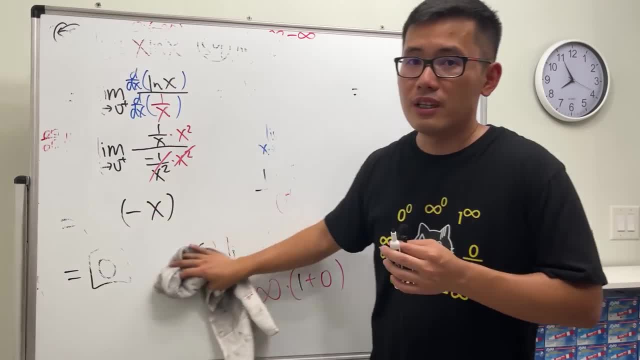 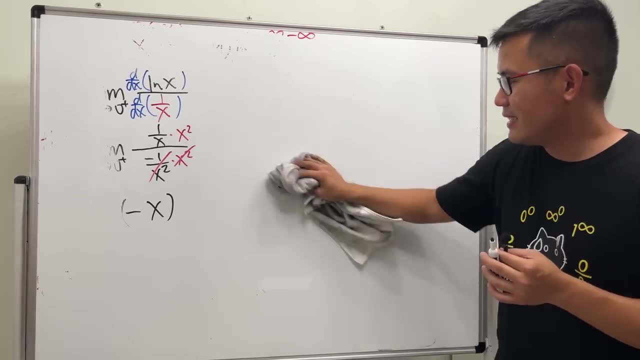 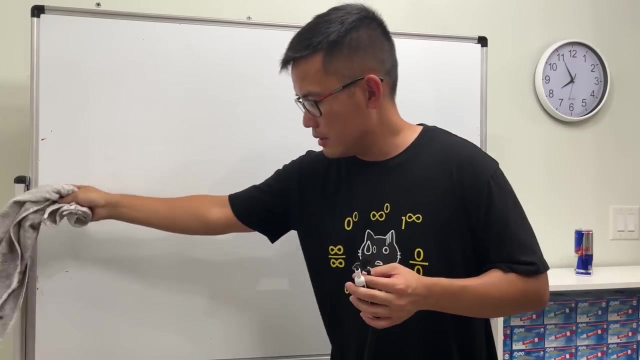 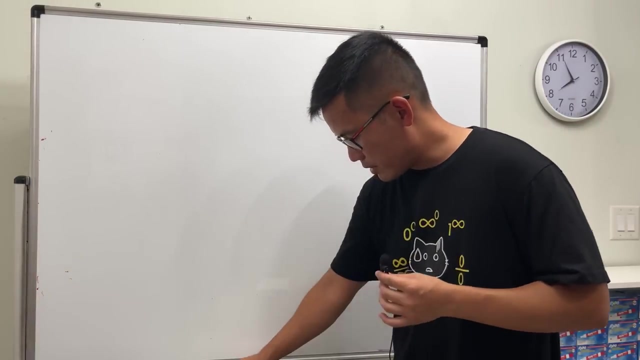 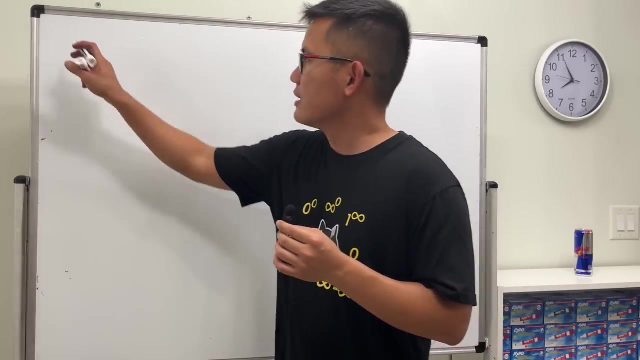 Yeah, You never know what you are going to get. Yeah, The limit is just like a box of chocolate. Yeah, Number 60.. I want to say 67, but no, not yet. It's 0 plus. So I'm going to put the limit as x approaching 0 plus. 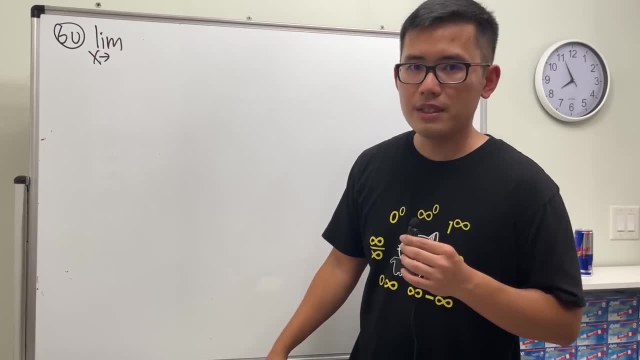 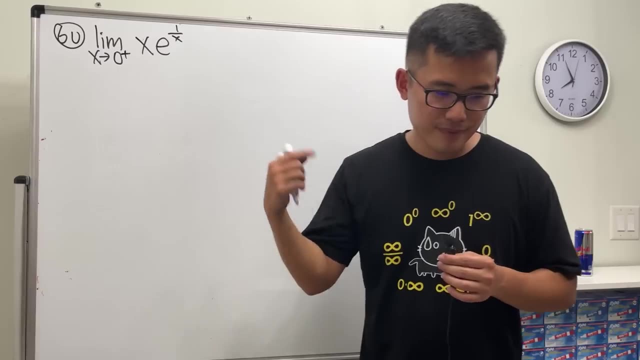 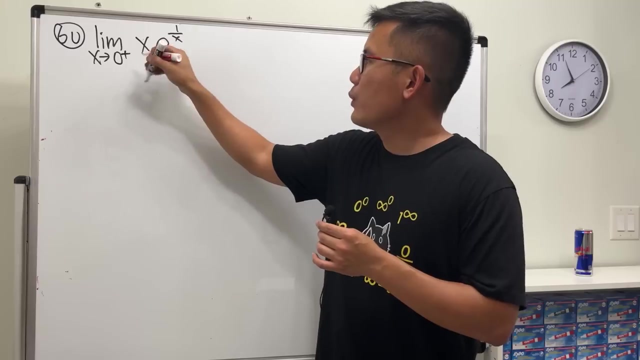 Yeah, Of course. Who came up with all this question? All right, If we put 0 plus into here and here check this out, We will end up with 0 times 1 over 0 plus is infinity. E to the infinity is infinity. 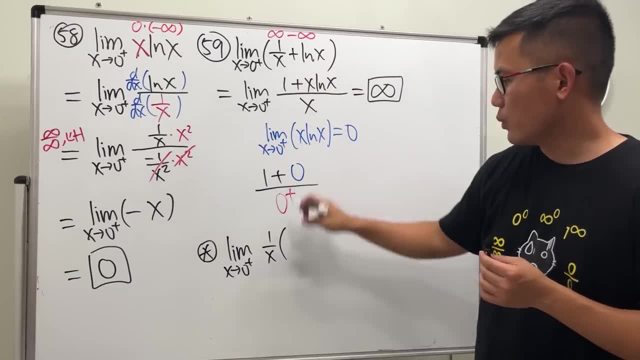 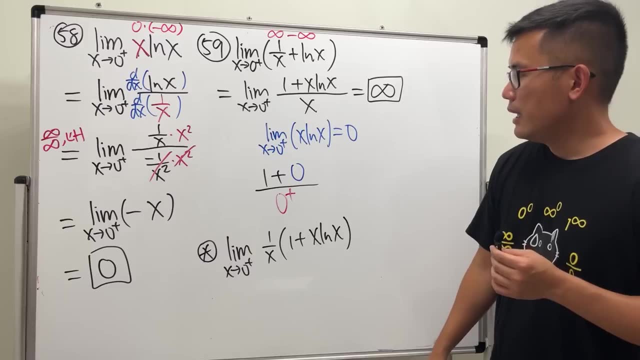 0 plus and then factor out the 1 over X and you will get 1 plus. if you factor 1 over X is like X times L and X, right, and it's pretty much like this, but like another look and you will see if you put. 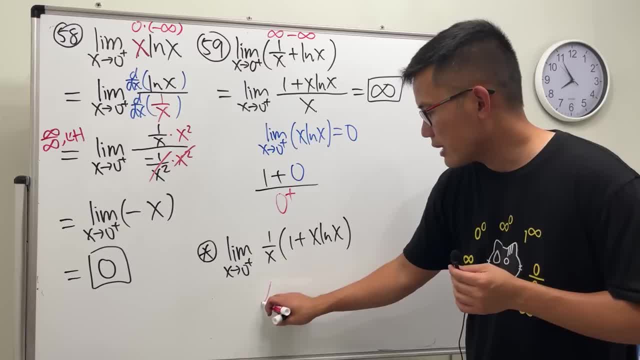 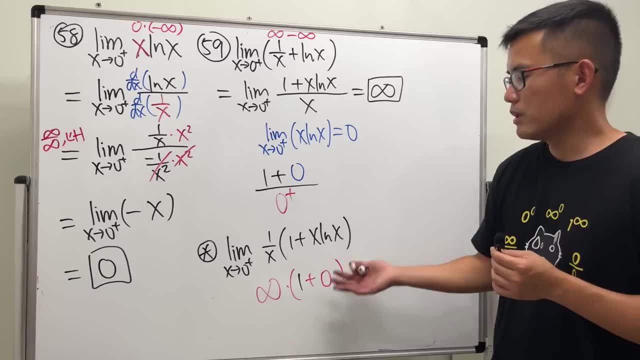 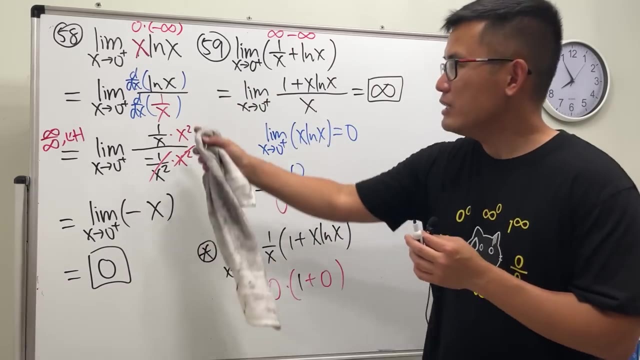 0 plus in here. this part is positive infinity, but this is 0. it's just like 1 plus 0, so infinity times 1 is infinity. yeah, so another way to look at it. but thanks to this part, imagine if this right here turns out to be negative: 1. 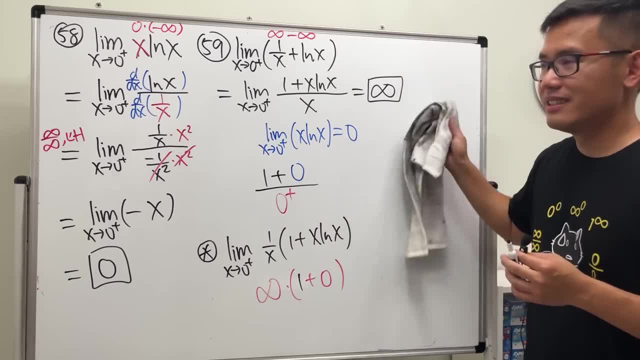 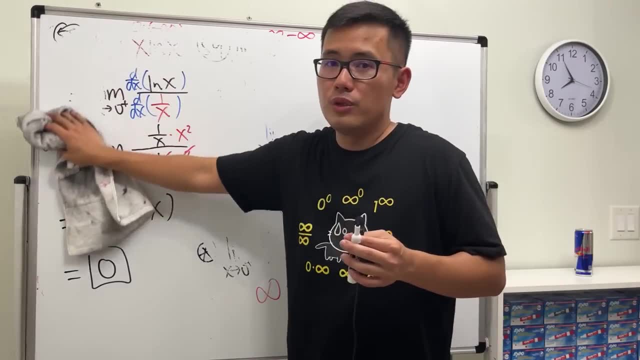 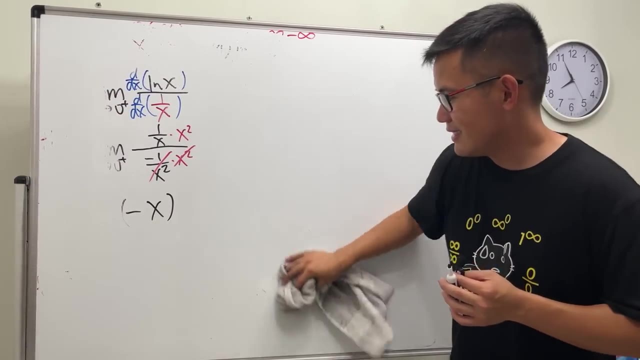 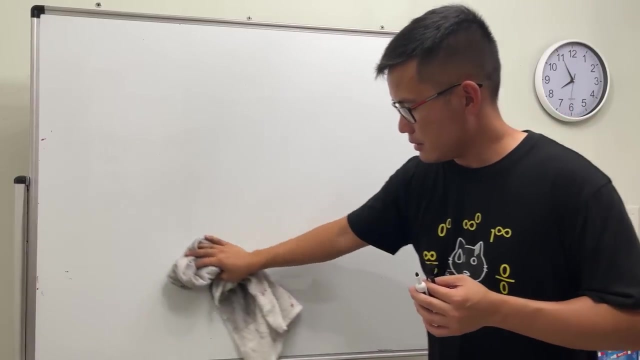 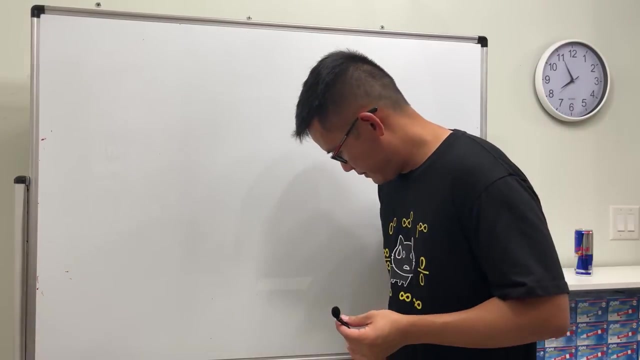 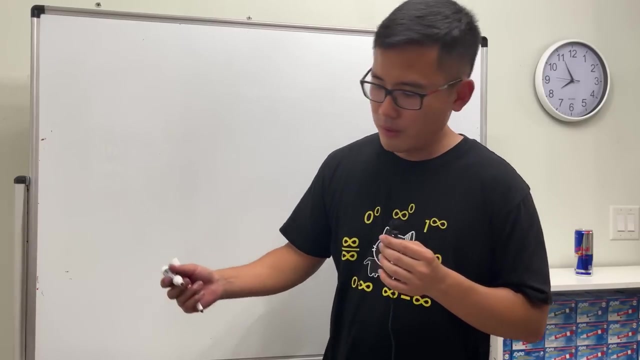 then this question will be hard to it, but it's not. and you see, infinity minus infinity gives us infinity. yeah, you'll never know, but you are going to get. yeah, doing limits is just like a box of chocolate. yeah, number 60. I want to say 67, but I know not yet. 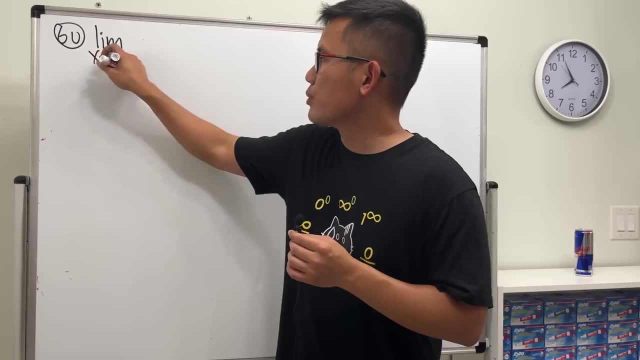 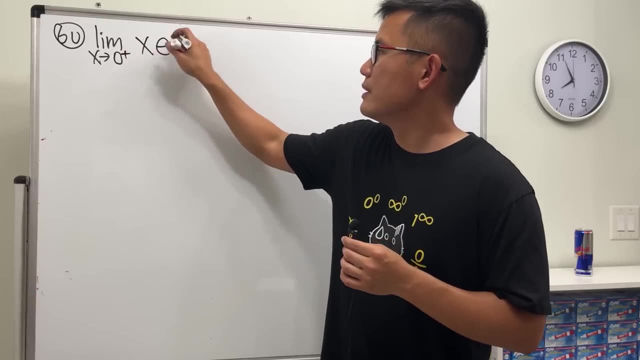 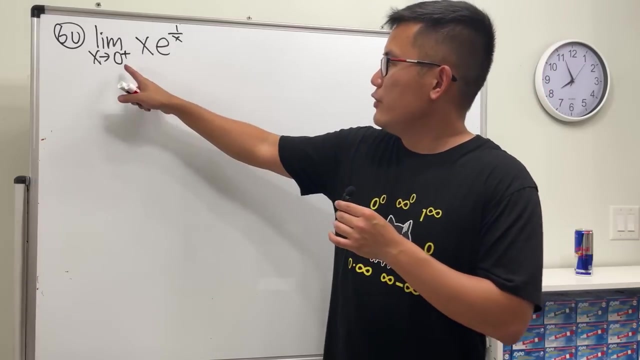 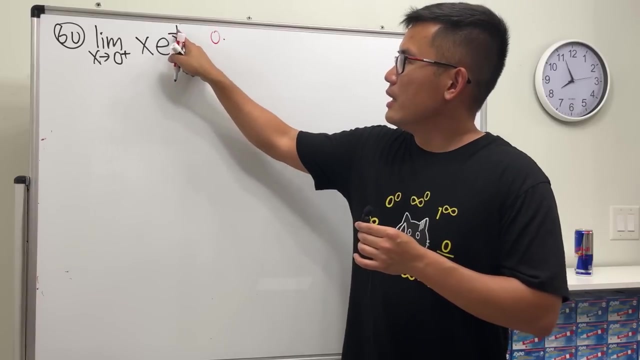 limit as X approaching 0 plus. yeah, of course. who came up with all this question? all right, if we put 0 plus into here and here check this out, we will end up with us 0 times 1 over 0 plus is infinity. e to the infinity is. 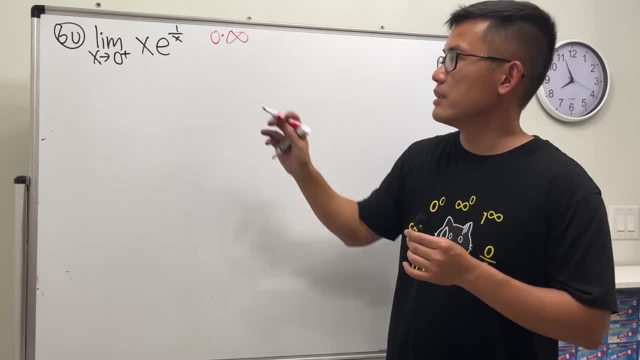 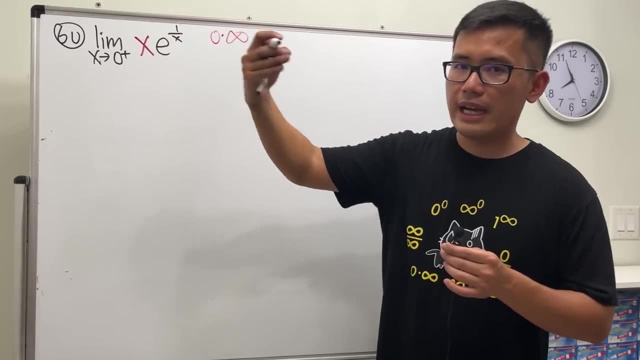 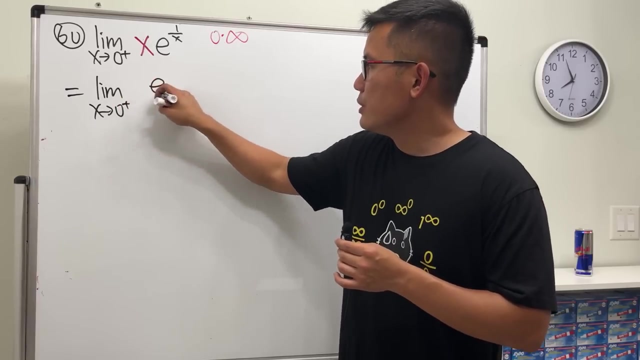 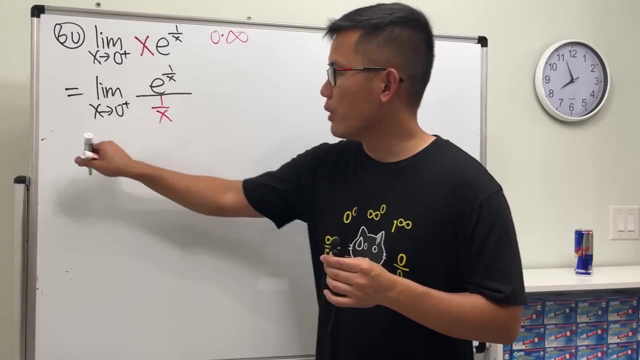 infinity. so this is 0 times infinity equals infinity, and now we use the final one. so we are gonna put 0 right here, but 0 is crossover. we are going to right here and we are gonna completely limit. we are going to ninguém. you've. 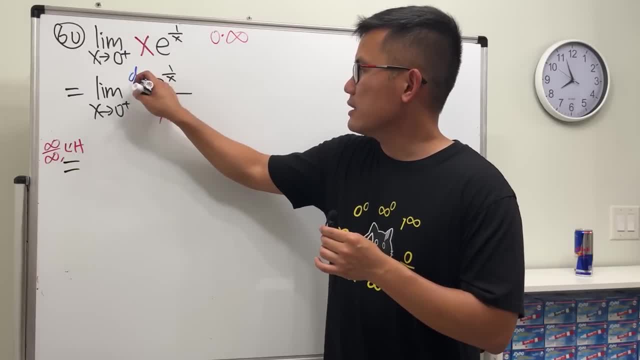 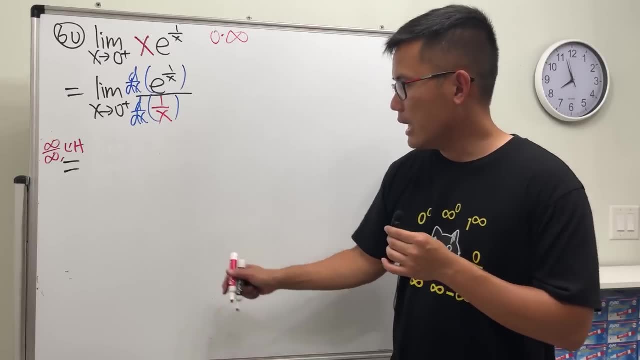 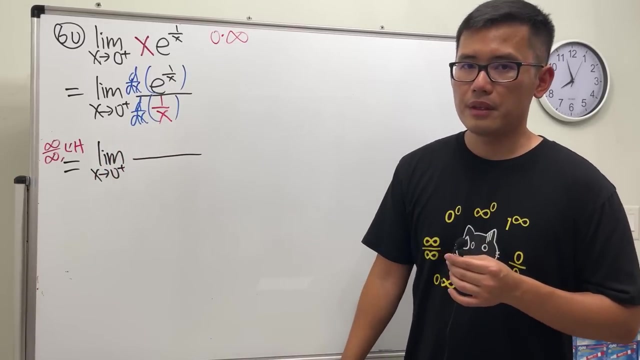 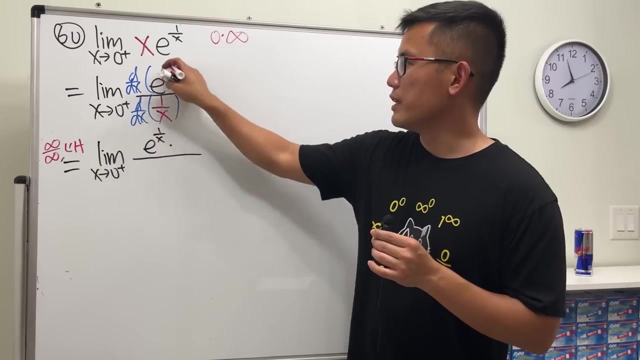 already, and then we can just say d, dx, d, dx. cool, now we have the limit as x approaching 0, plus what's the derivative e to the something? the answer is: you first repeat that e to the 1 over x and then you multiply by the derivative of the inside, because of the chain rule and the derivative. 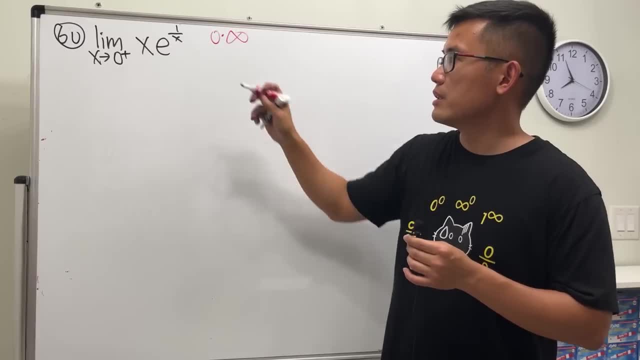 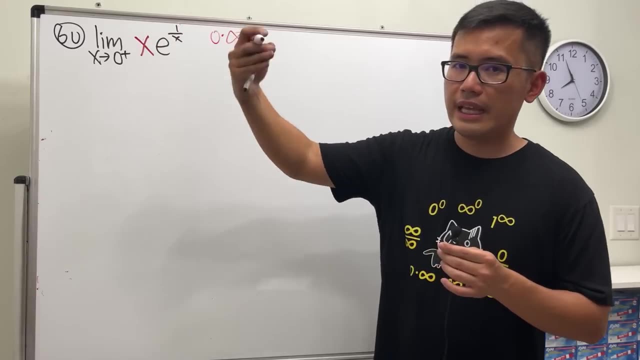 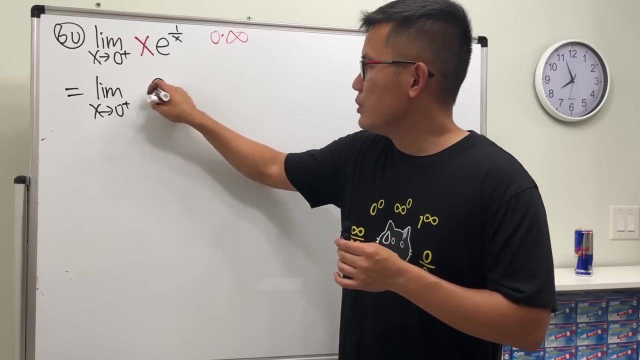 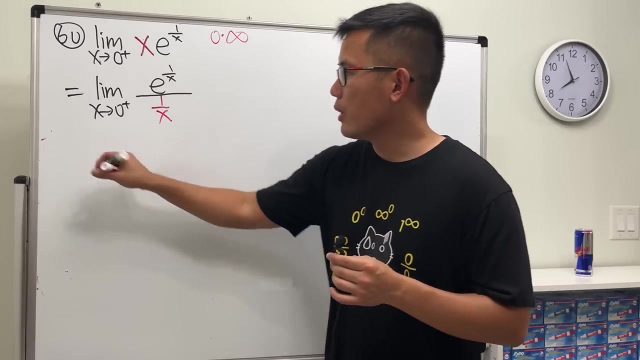 So this is 0 times infinity, zero times infinity situation. so we are going to do what we did earlier. here's the x. bring that down down. this right here is the limit as x approaching zero plus e to the one over x states on the top. but then we write this as one over x on the denominator and we will. 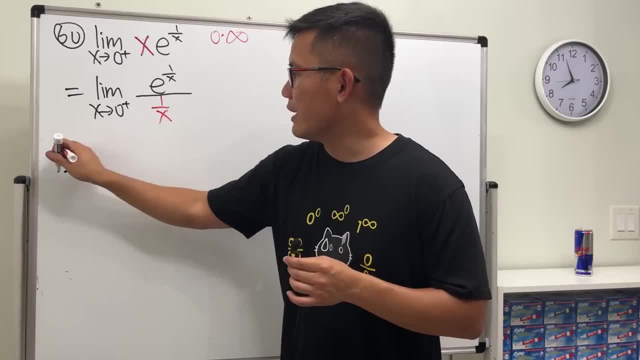 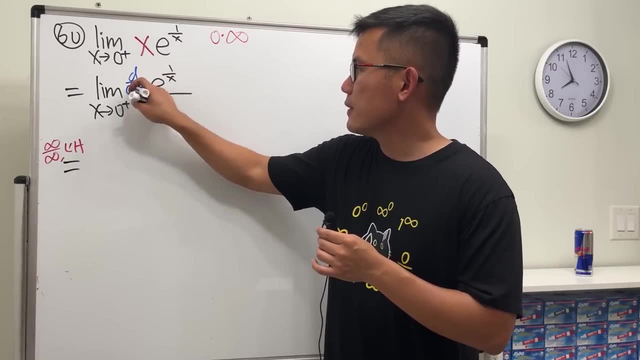 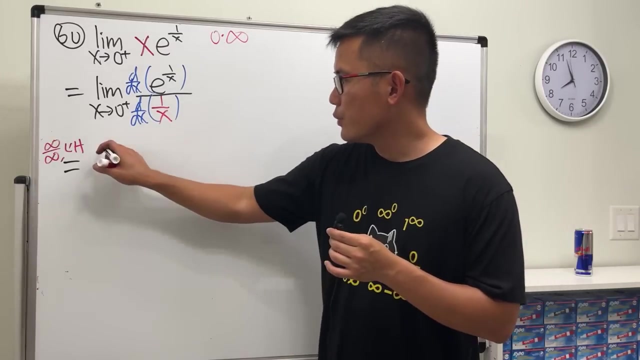 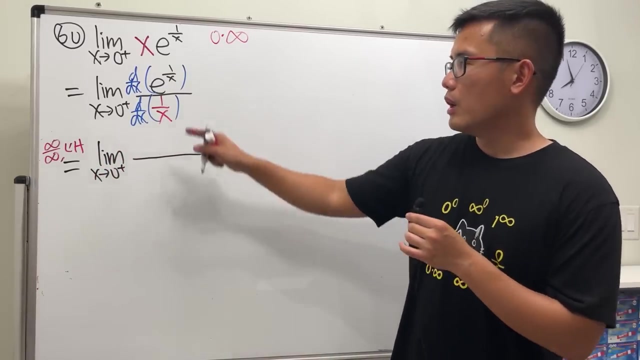 use the Lapito's rule, because now we have infinity over infinity, so it's Lapito's rule ready, and then we can just say d, dx, d, dx. cool, now we have the limit as x approaching zero, plus what's the derivative e to the something? the answer is: you first repeat that e to the one. 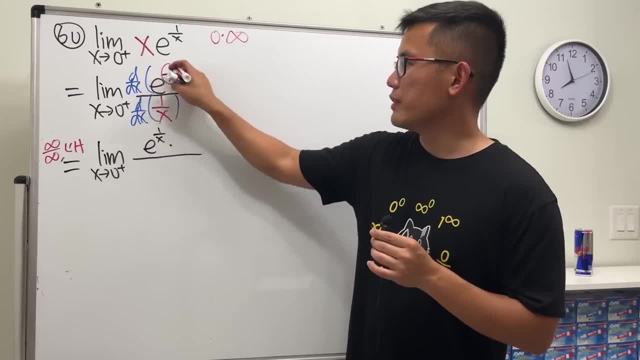 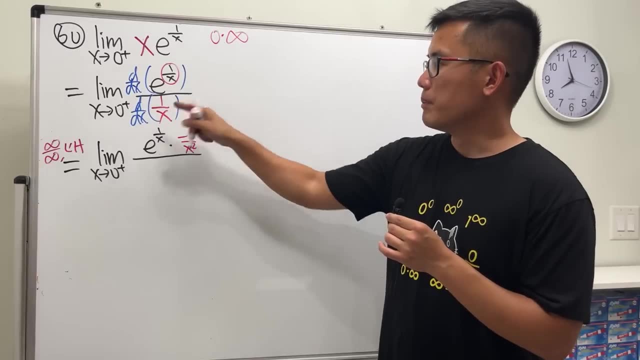 over x and then you multiply by e to the one over x, and then you multiply by e to the one over x and then you multiply by the derivative of the inside, because of the chain rule, and the derivative of that is negative. one over x square the bottom. when we differentiate that we also get negative one over. 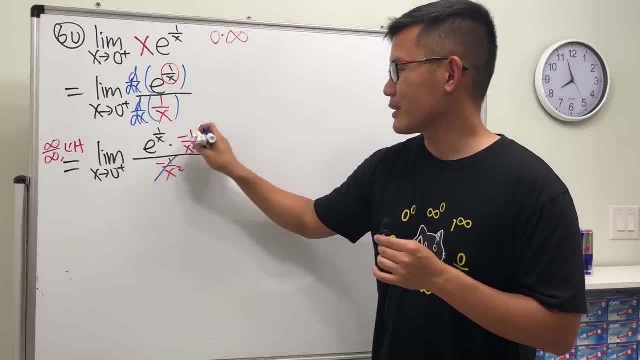 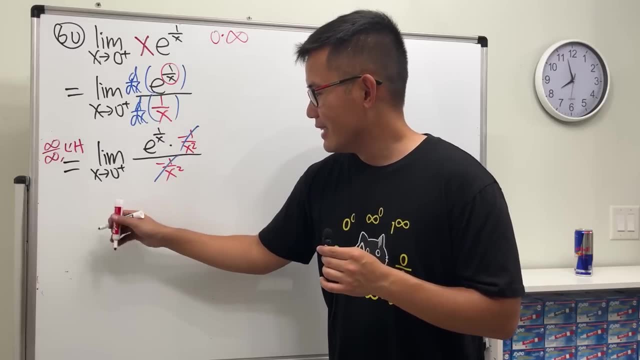 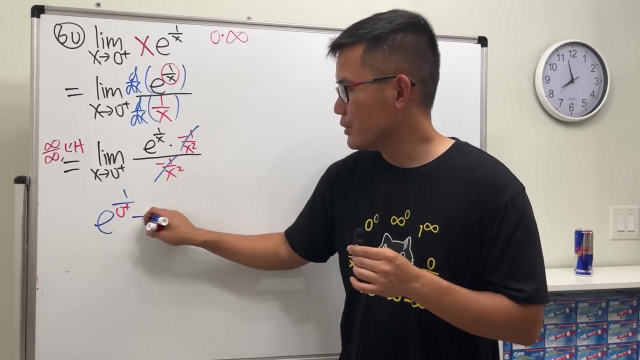 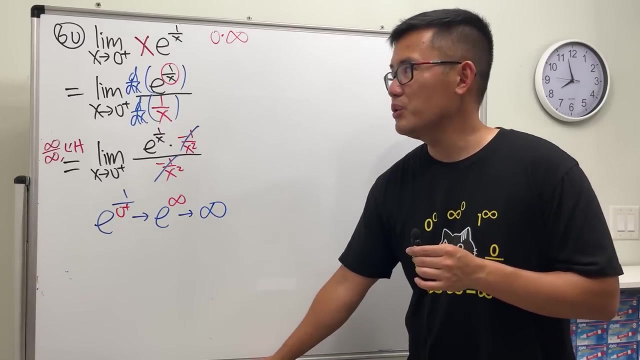 x square. let's cancel each other out completely. oh my god, check this out. when we put zero plus into here, now we get what we get this. this is now e to the one over zero plus, which is e to the infinity, which is infinity. told you, zero times, infinity is not always. 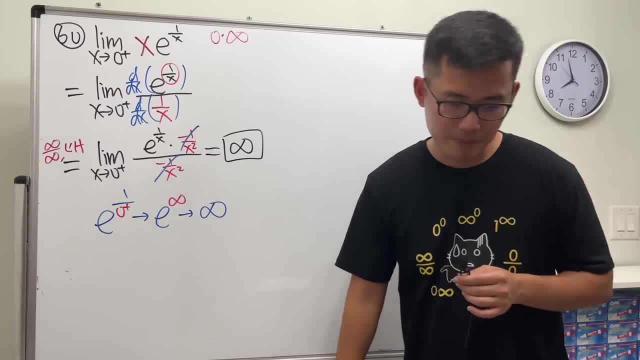 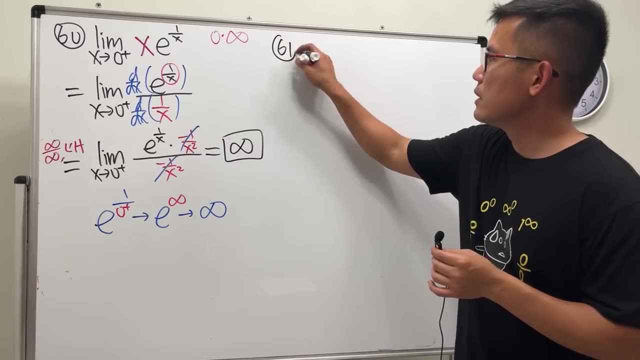 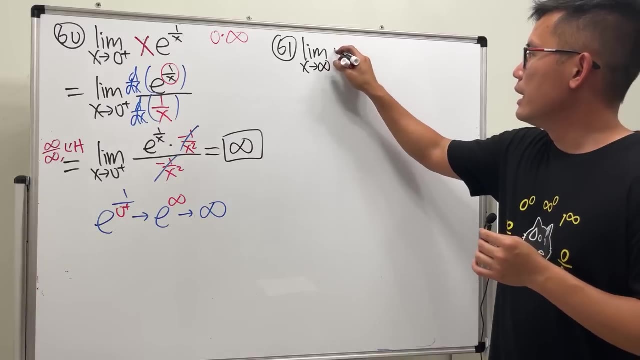 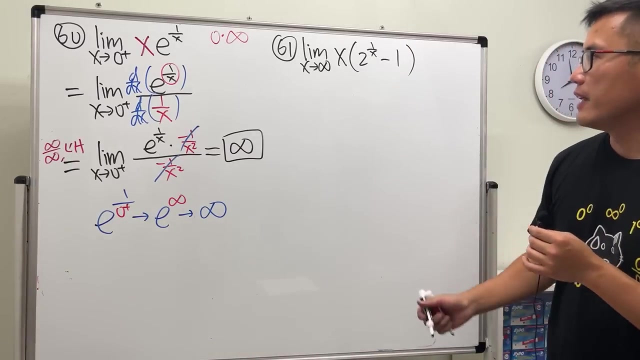 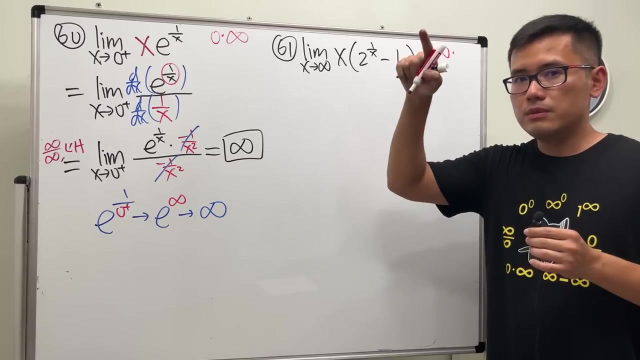 equal to zero. sometimes infinity can win too. all right, number 61 limits as x approaching infinity, x times two to the 1 over x minus one. all right, similar flavor this time now, if we put infinity to here, we get infinity times 1 over infinity 0. 2 to the 0 is 1, 1 minus 1, 0, so infinity times 0. so do the same thing. 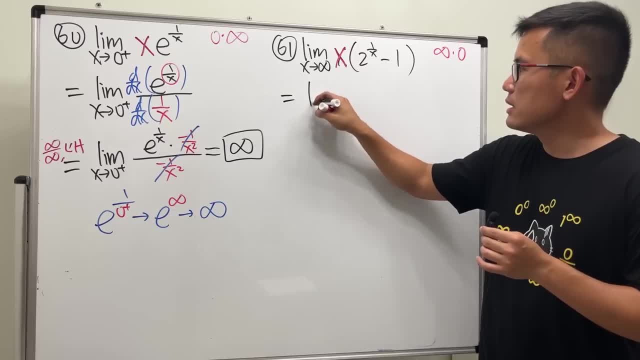 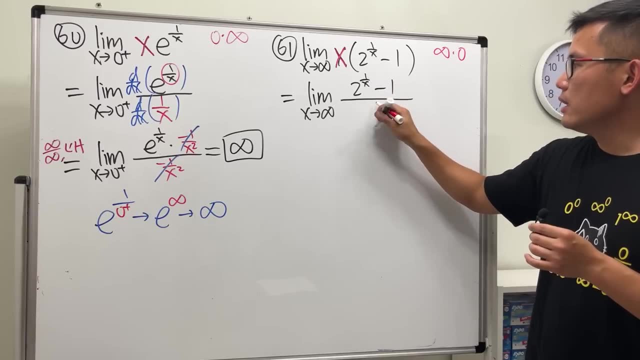 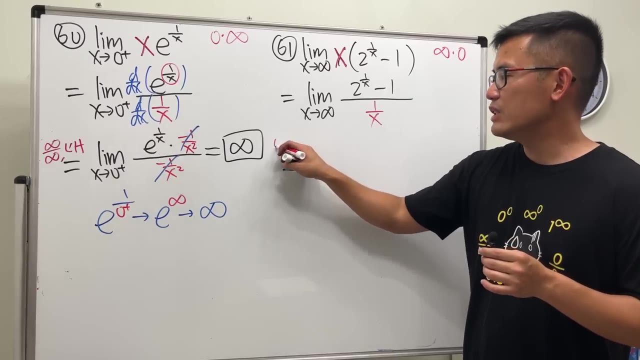 put this x down down. so we're looking at this as limit, as x approaching infinity. here we get 2 to the 1 over x, minus 1 over 1 over x, and you know it. we can use l'Hopital's rule, because this time we get 0 over 0. you can use l'Hopital's rule. 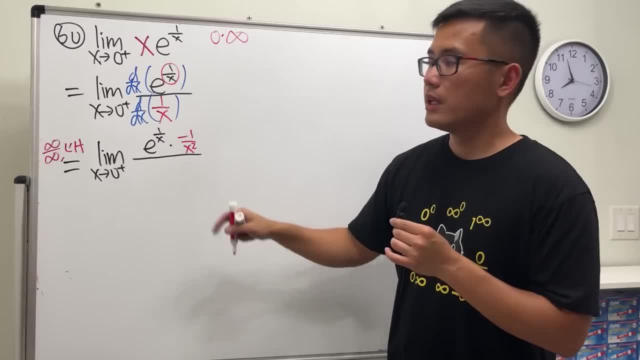 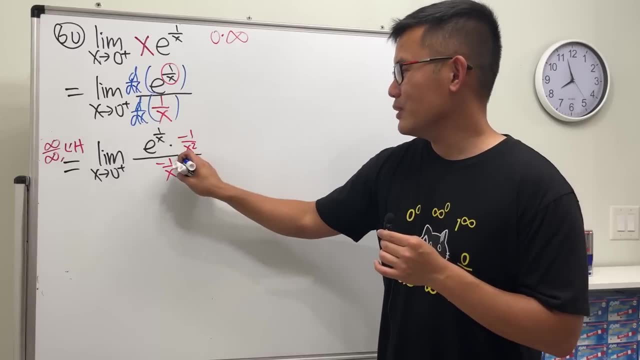 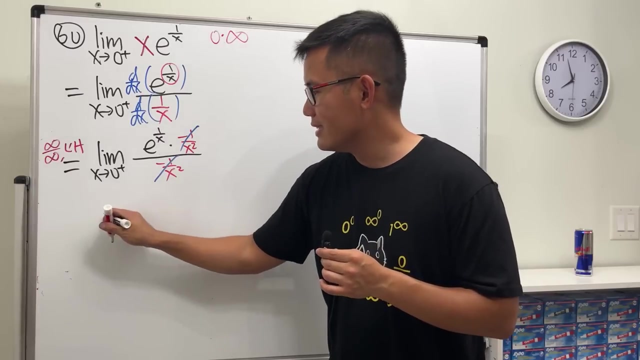 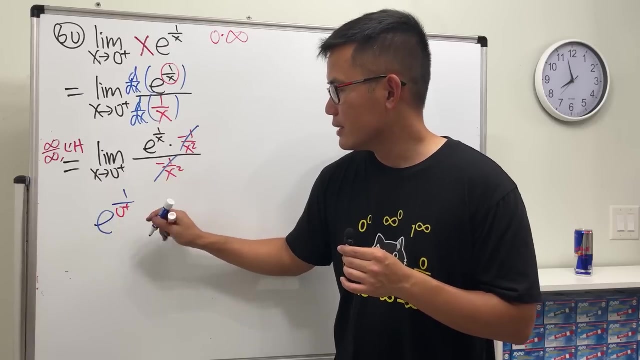 of that is negative 1 over x square- the bottom. when we differentiate that, we also get negative 1 over x square. let's cancel it out completely. oh my god, check this out. when we put 0 plus into here, now we get what we get this: this is now e to the 1 over 0 plus, which is e to the infinity. 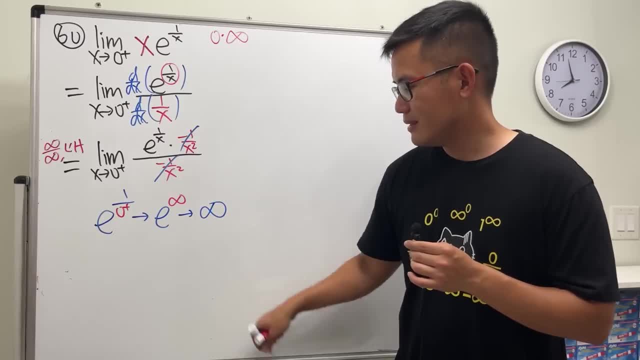 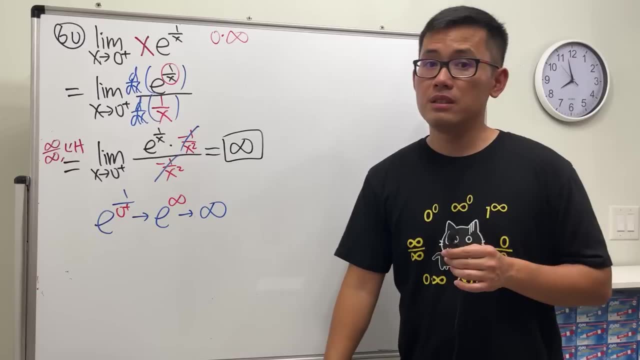 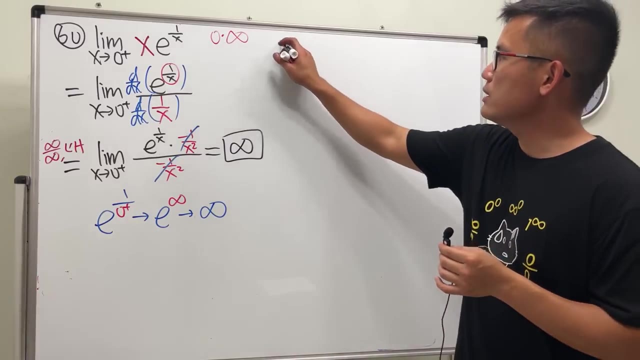 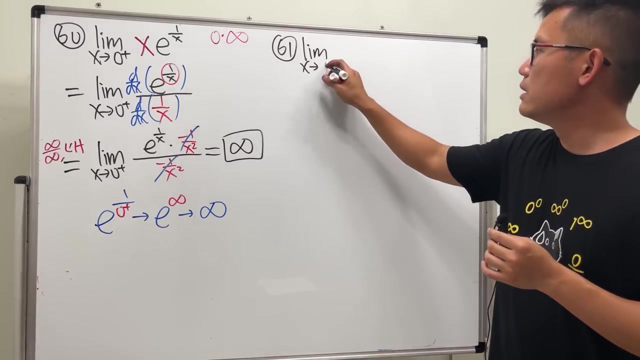 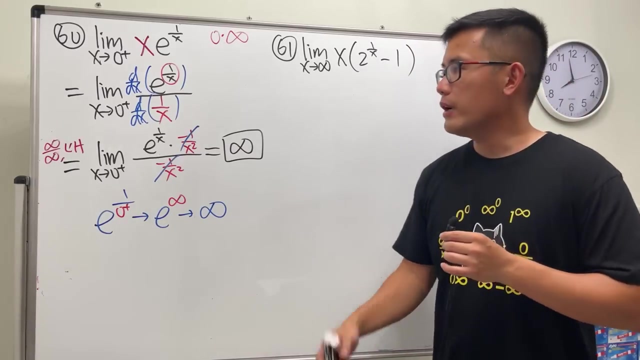 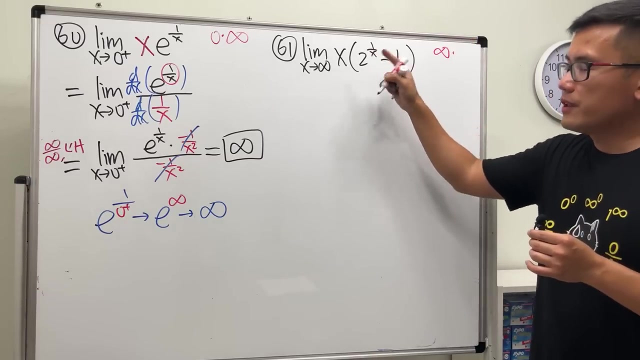 which is infinity, told you, 0 times. infinity is not always equal to 0. sometimes infinity can win too. okay, infinity, all right. number 61 limit as x approaching infinity, x times 2 to the 1 over x minus 1. all right. similar flavor this time. now, if we put infinity to here, we get infinity times 1 over infinity 0. 2 to the 0 is 1. 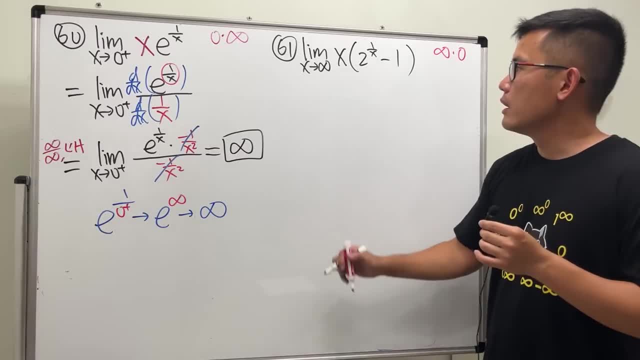 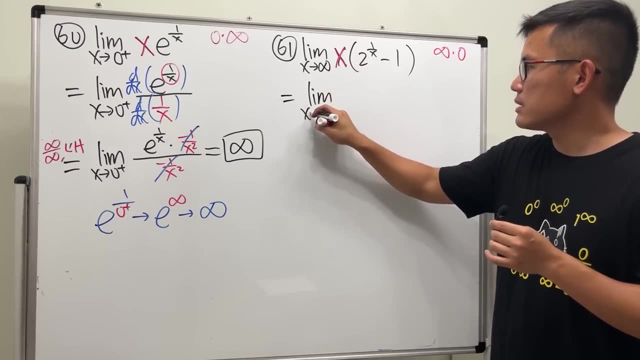 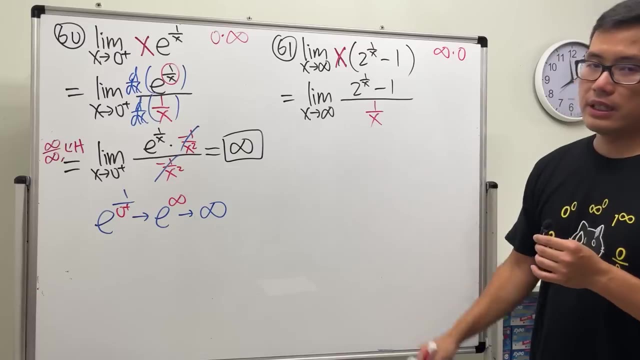 1 minus 1 is 0, so infinity times 0. so do the same thing, put this x down down. so we're looking at this as limit, as x approaching infinity. here we get 2 to the 1 over x minus 1 over 1 over x, and you know. 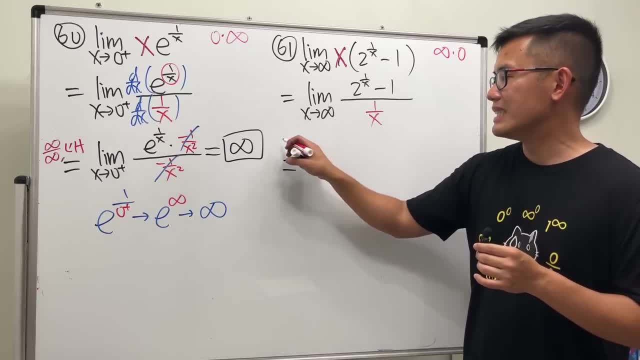 it. we can use lopito's rule, because this time we're going to put this x down down, so we're going to be going a little big enough. this time we get 0 over 0. you can use lopito's rule, so, ladies and. 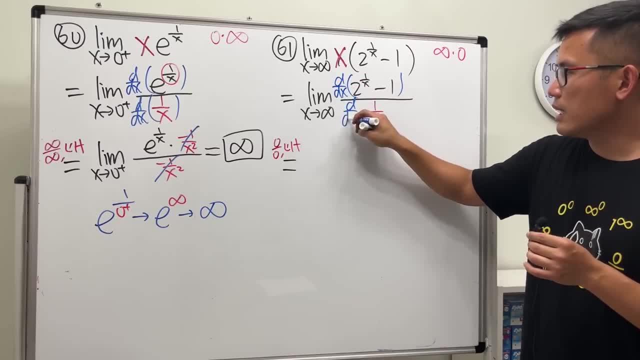 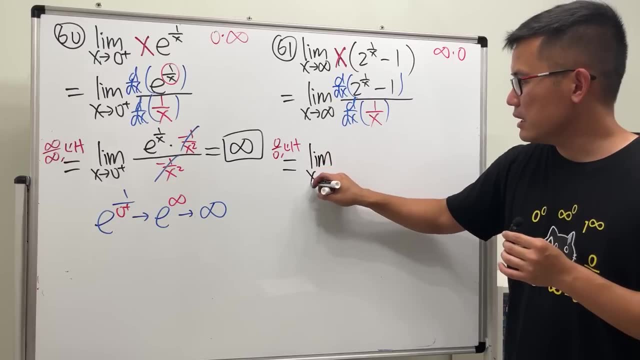 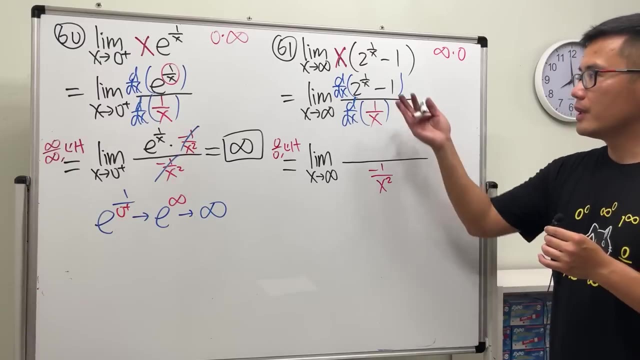 gentlemen, d dx here. d dx just means that we are going to take the derivative. so here we have the limit as x approaching infinity. the bottom: here we get negative 1 over x square. how about the top? what's the derivative of 2 to d to the? 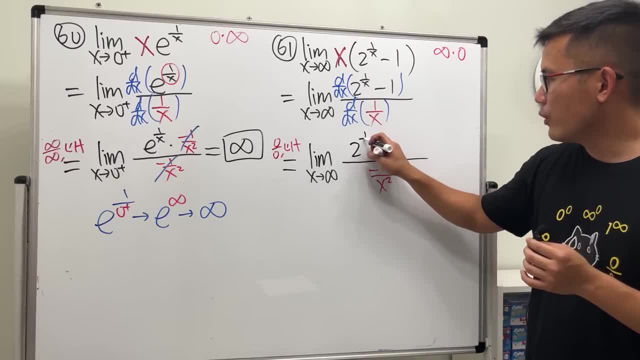 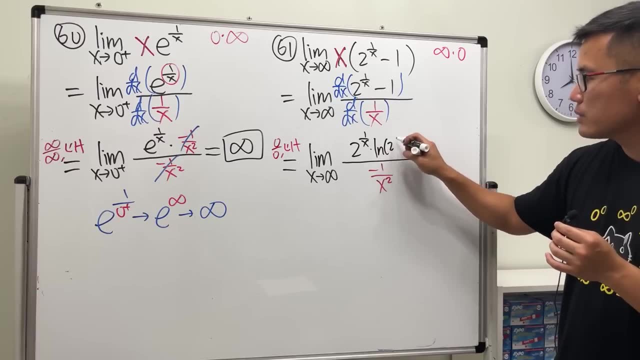 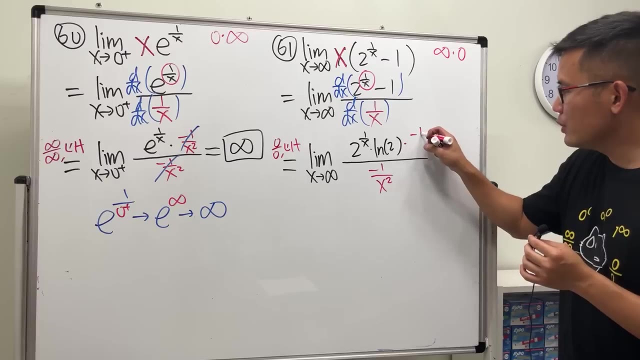 Let me tell you. it first repeats 2 to the 1 over x, but because the base right here is a 2, it's not e, so we will multiply by ln of the base which is 2, and then we multiply by the derivative of that, because of the chain rule, which is negative: 1 over x, squared. 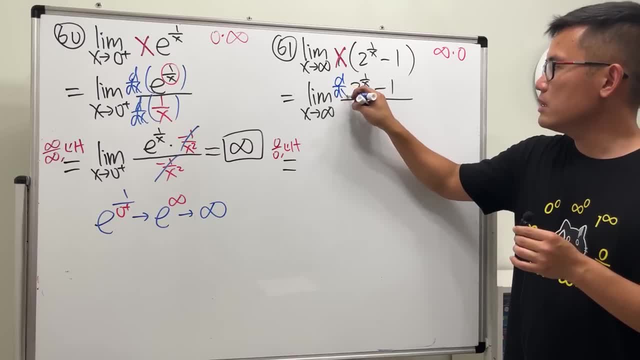 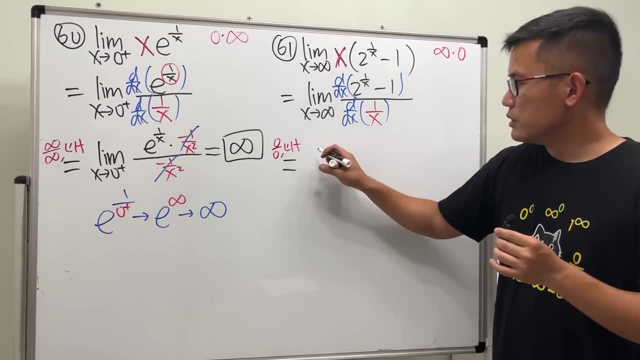 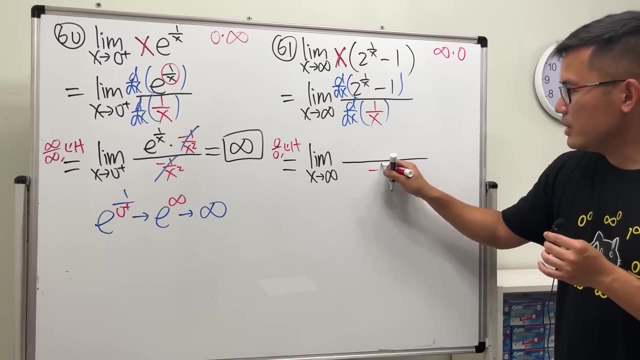 so, ladies and gentlemen, d dx here. d dx just means that we are going to take the derivative. so here we have the limit as x approaching infinity. the bottom: here we get negative 1 over x square. how about the top? what's the derivative? 2 to the 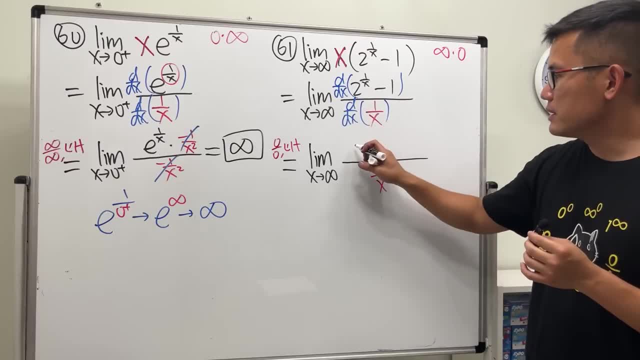 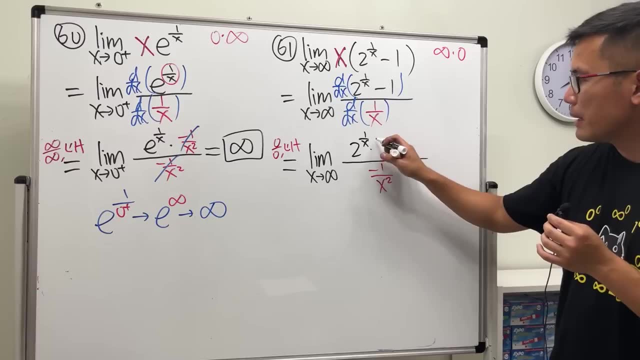 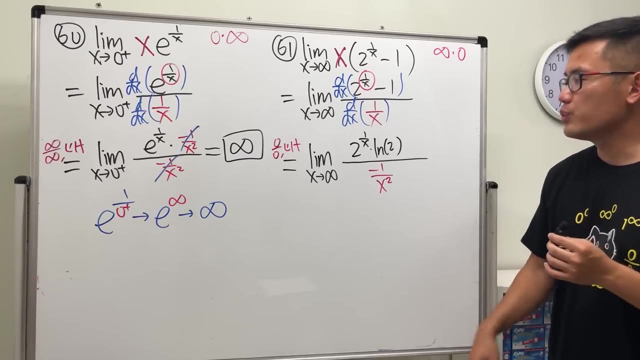 d manifestation. David, let me tell you. it first repeats 2 to the 1 over x. but because the base right here is a, 2, it's not e, so we will multiply by ln of the base which is 2, and then we multiply by the derivative of that because of the change. 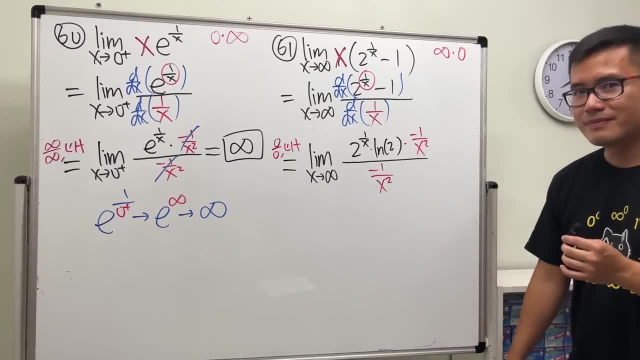 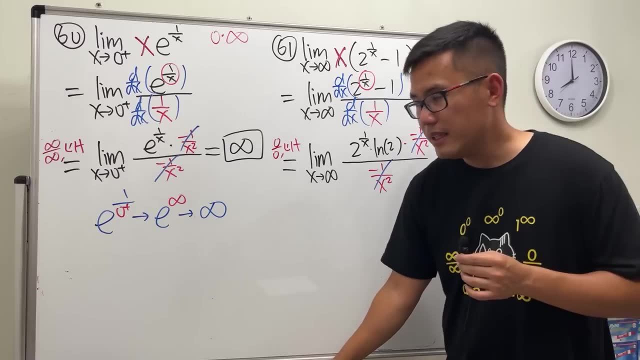 rule which is negative, 1 over x square, the derivative of minus 1 is 0, that's an d DX. and then you will say it's 3.7 minus 1 over x square, won't be able more. and then we see that this and that cancel. and when we put infinity to here, 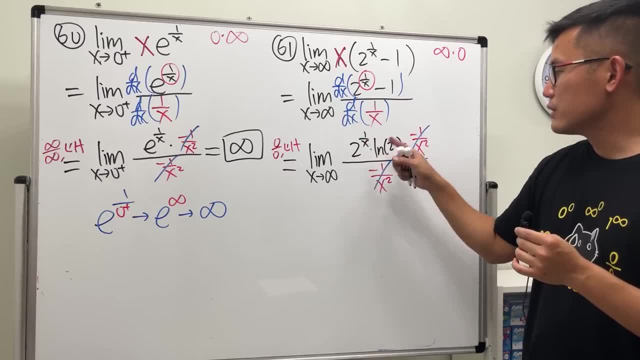 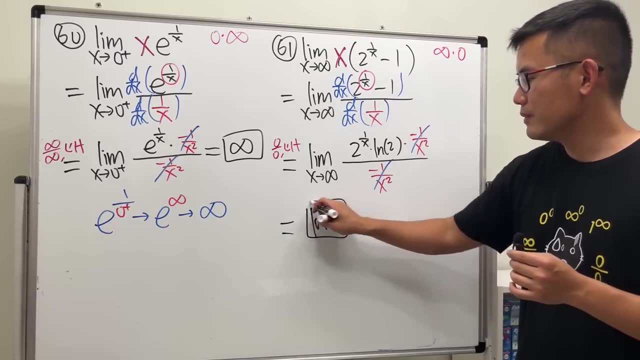 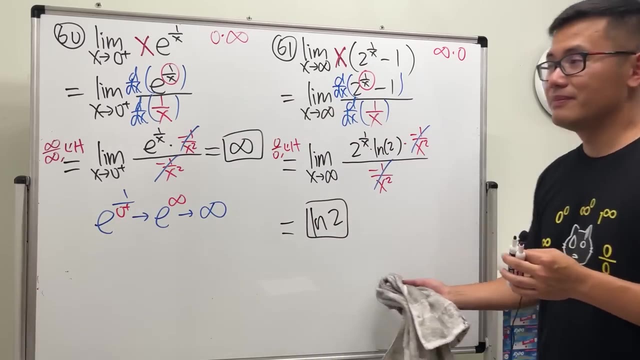 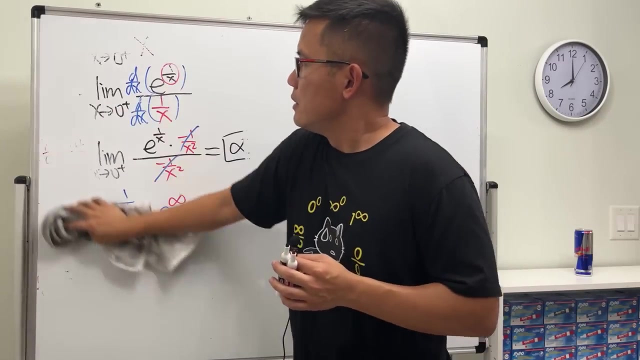 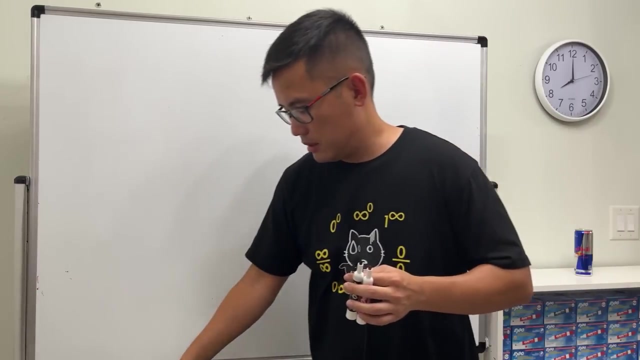 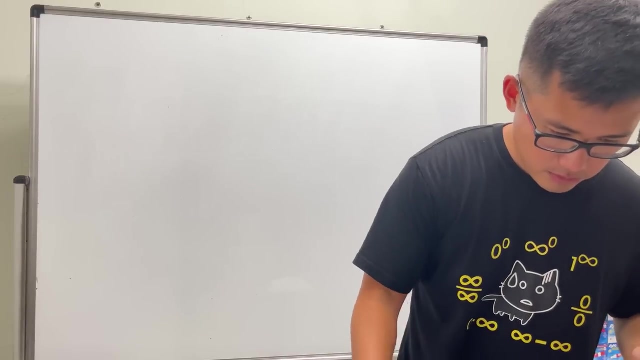 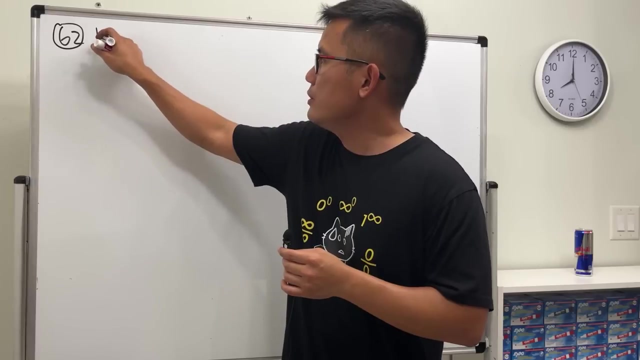 1 over infinity is 0,. 2 to 0 is 1, so 0 times infinity gives us ln2, told you, 0 times infinity. you can get a lot of different things in indeterminate forms. crazy huh. number 62 limit as X approaching. 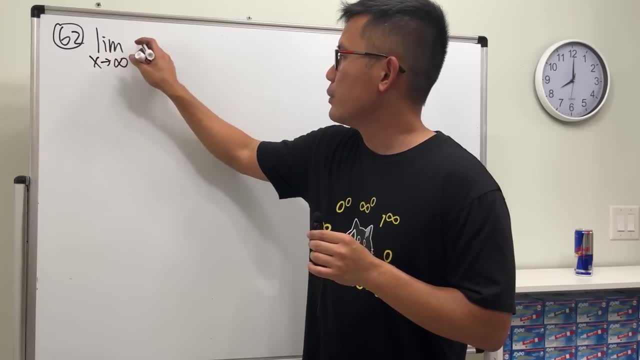 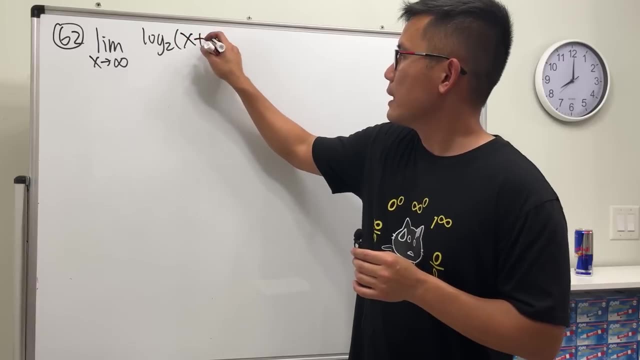 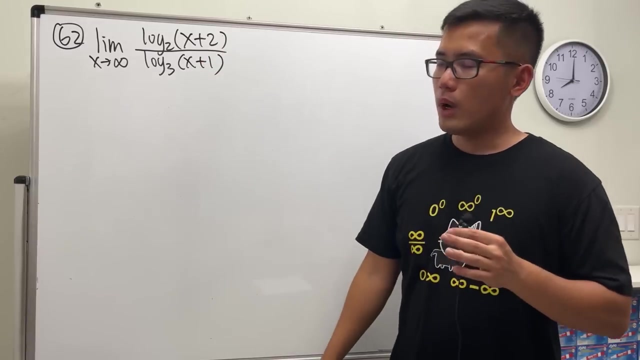 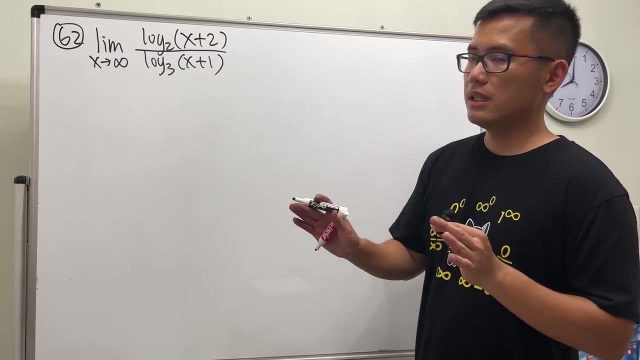 infinity. and then we have log base 2 of X plus 2 over log base 3 of X plus 1. okay, we get infinity over infinity. so let's just get it out of way and let's just go ahead and use the L'Hospital's rule, because this is an 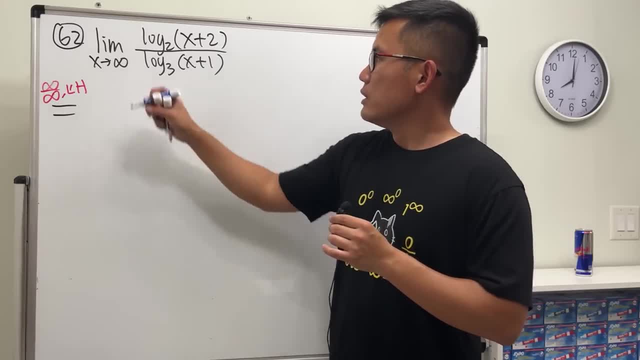 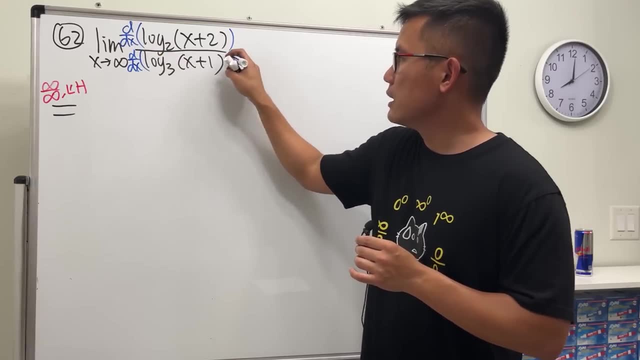 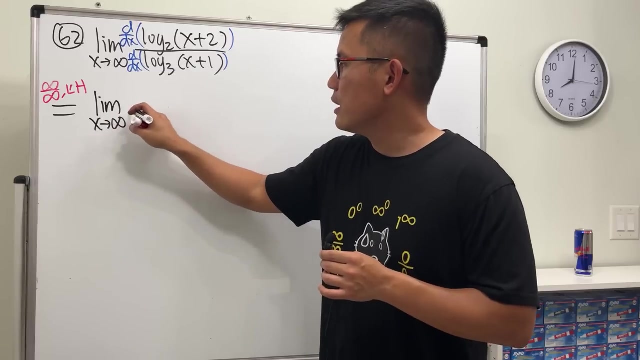 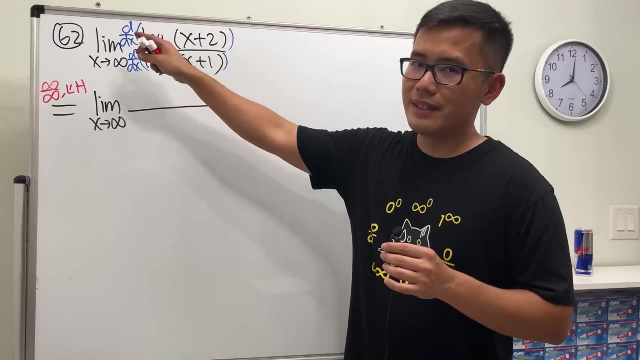 infinity form, infinity over infinity situation. so everybody's favorite ddx, ddx. here is the limit as X approaching infinity. so how do we differentiate? this, though, we'll tell you when we have ln. so when we have log of 2, right log base, 2 you just put. 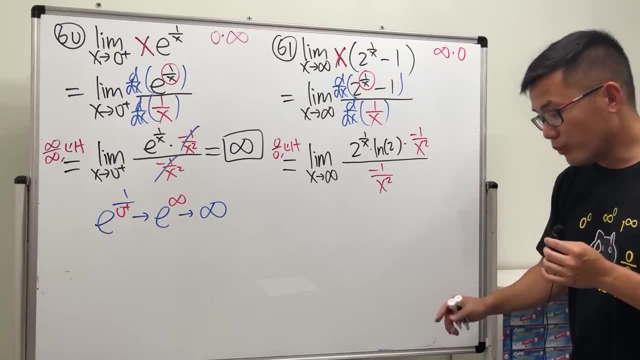 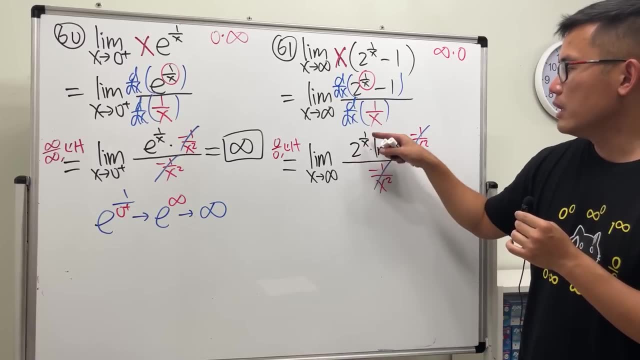 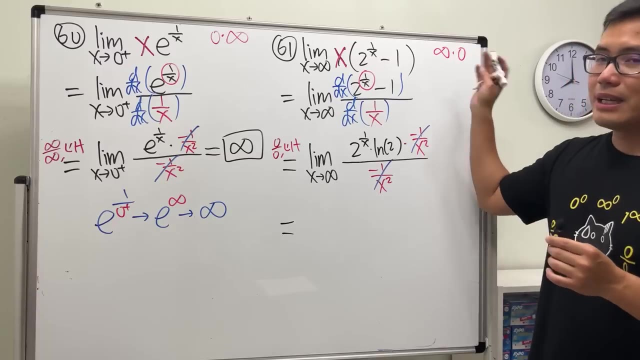 The derivative of minus 1 is 0, so no more. and then we see that this and that cancel, and when we put infinity to here, 1 over infinity is 0,, 2 to the 0 is 1, so all in all, 0 times infinity gives us ln2.. 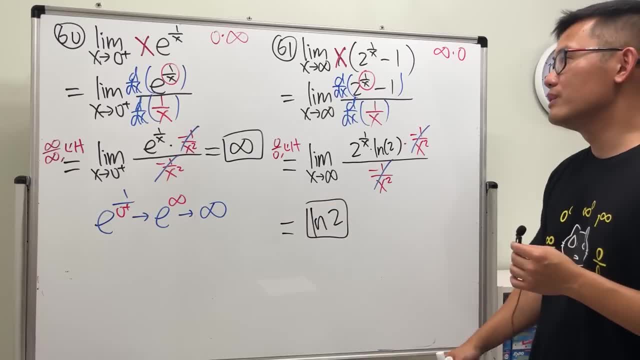 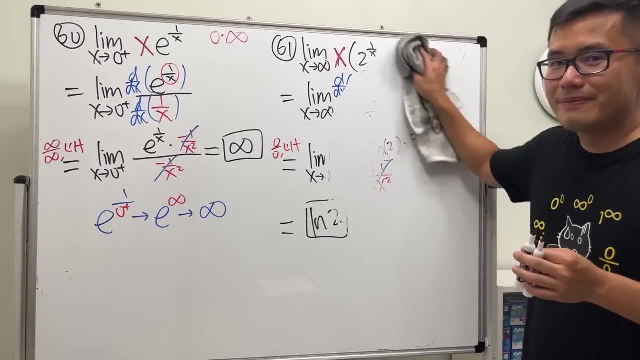 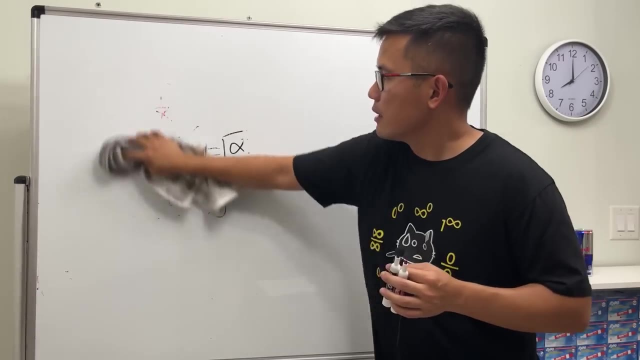 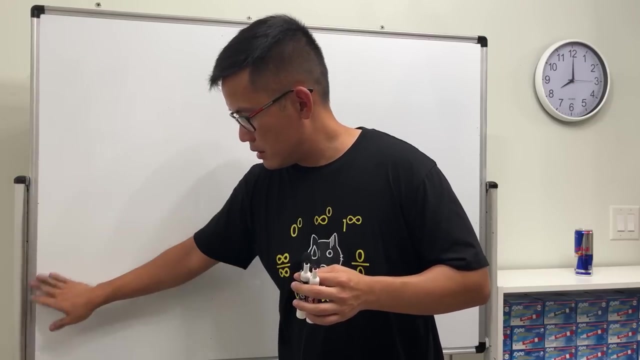 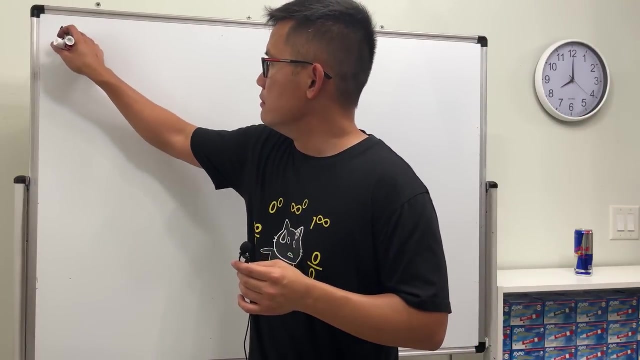 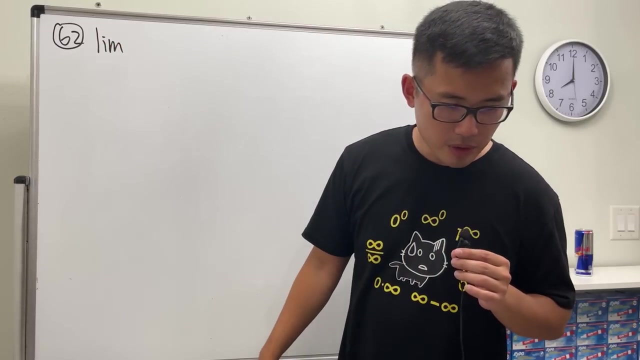 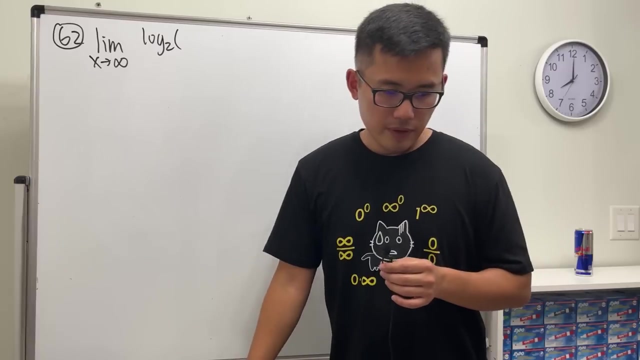 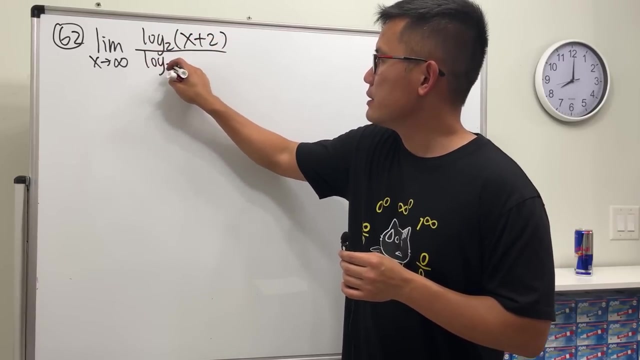 So I told you, 0 times infinity. you can get a lot of different things in determinant forms: Crazy huh, Number 62, limit as x approaching infinity, And then we have log base 2 of x plus 2 over log base 3 of x plus 1.. 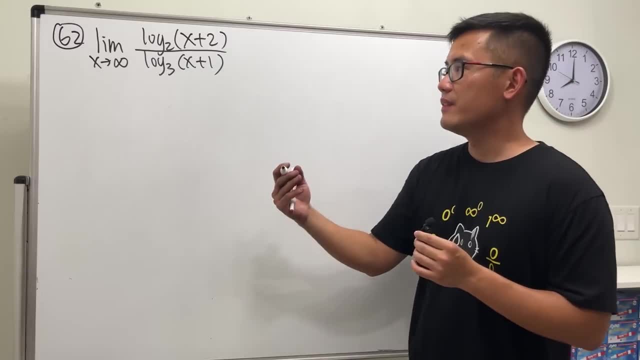 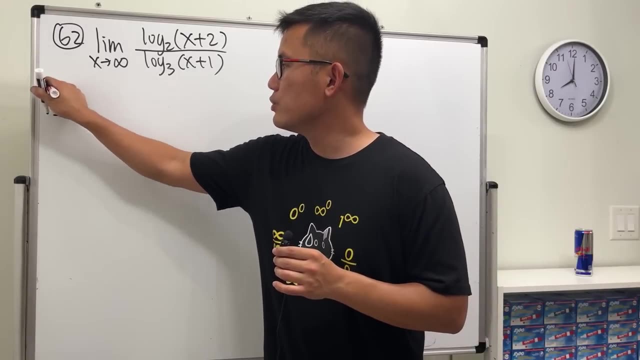 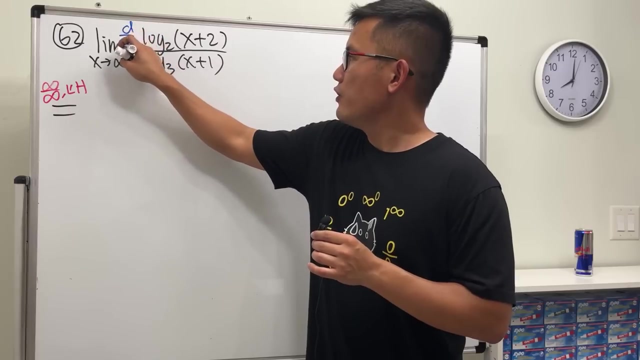 Wow, Okay, we get infinity over infinity. So let's just get that out of the way and let's just go ahead and use L'Hopital's rule, because this is an infinity over infinity situation. So everybody's favorite: ddx, ddx. 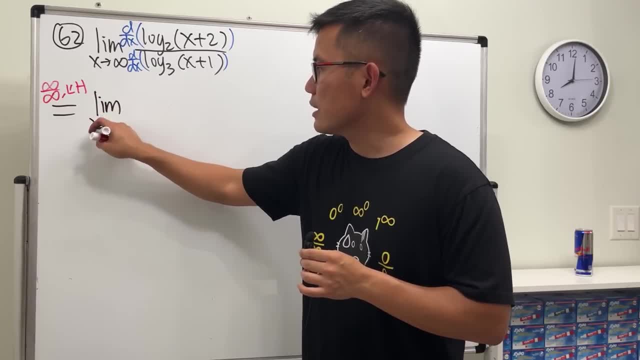 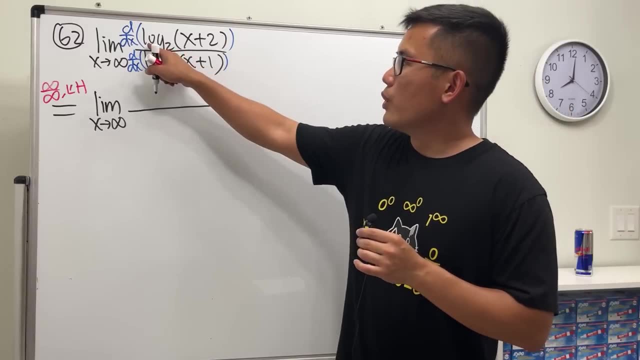 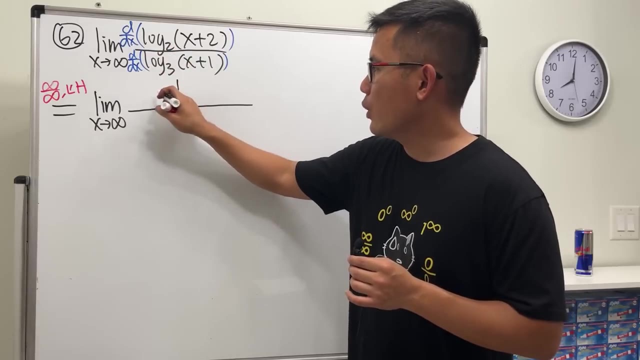 Here is the limit as x approaching infinity. So how do we differentiate this, though? We'll tell you When we have ln. so when we have log of 2, right log, base 2, you just put this on the bottom first, so you have 1 over x plus 2.. 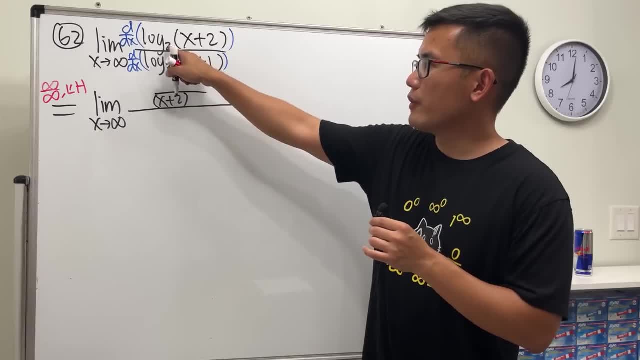 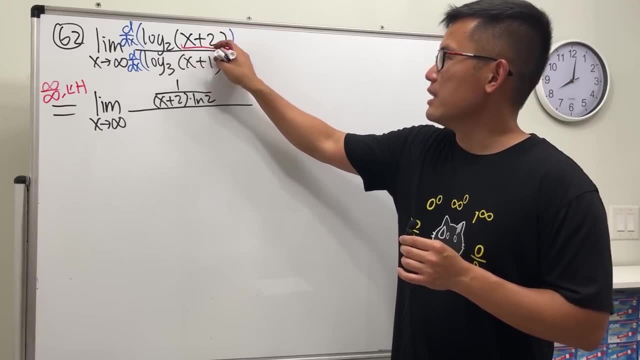 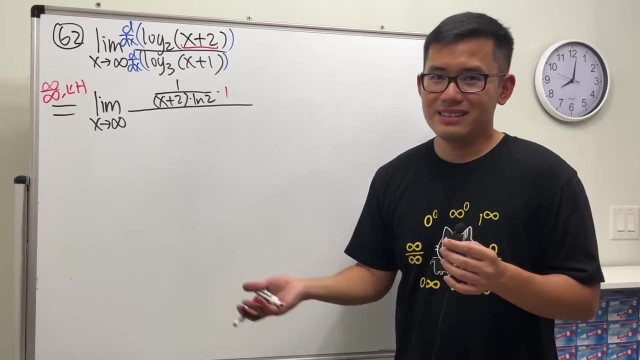 But you also multiply by ln of that base. so you multiply by ln2, okay, And then you check the derivative of the inside. but the derivative of x plus 2 is just 1.. So if you forget the chain rule, you know you're lucky just because multiply by 1 doesn't matter. 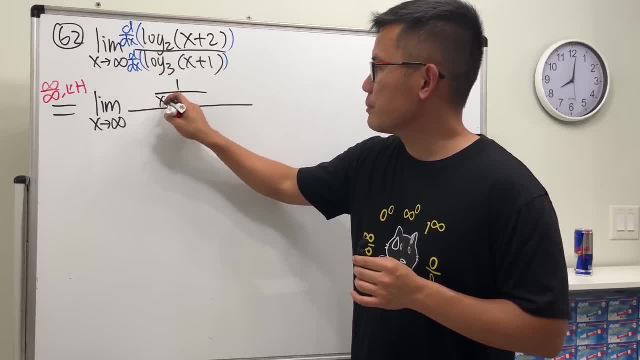 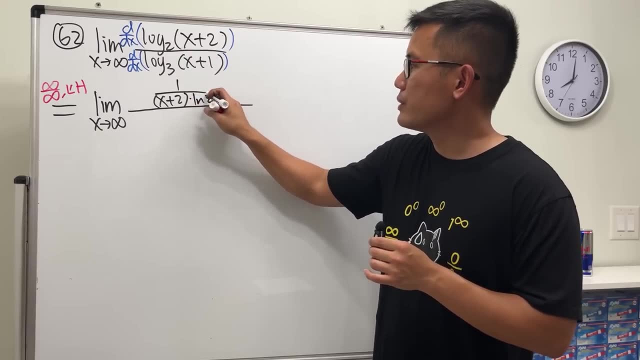 this on the bottom first, so you have 1 over LN, but then we have positive 0. that remember when we have 0 over x plus 2. you need to veβ into that thing. that's very simple. also, you multiply by L, this time. 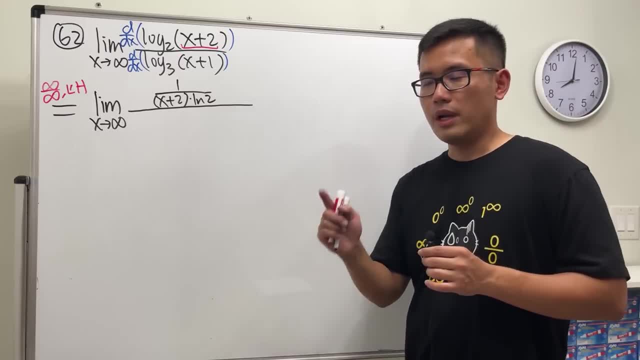 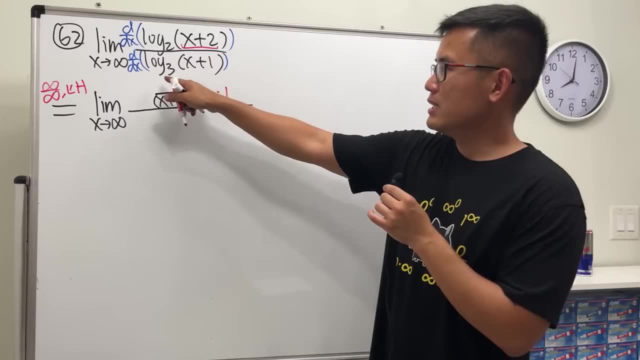 Okay, and then you check he derivative of the inside, but the derivative X plus 2 is just 1. so if you forget a chain rule, you know you're lucky just because multiple 1 doesn't matter. alright, let's practice this again. the review positive log, base 3. 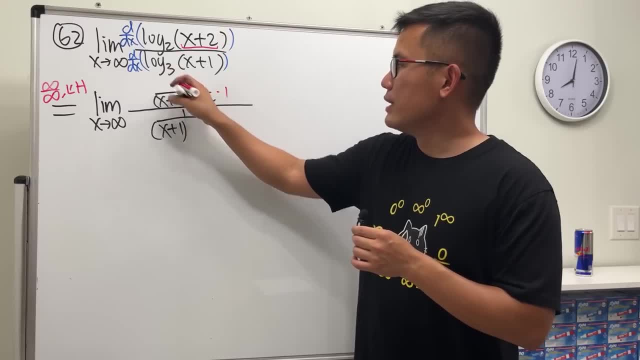 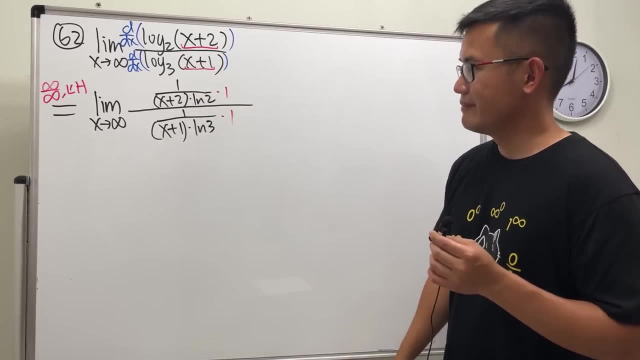 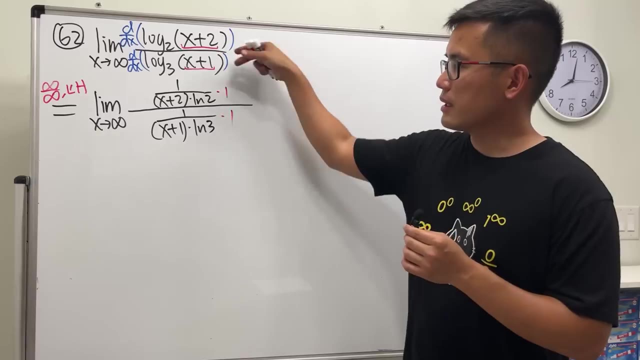 x plus 1 times ln, 3, okay. and then multiply by the derivative of this, which is also 1. cool, now we want the x to be going to infinity, but let's just put this on the top. so on all, we are looking at the limit. 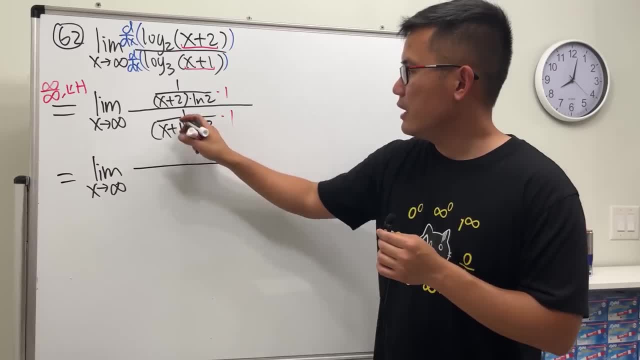 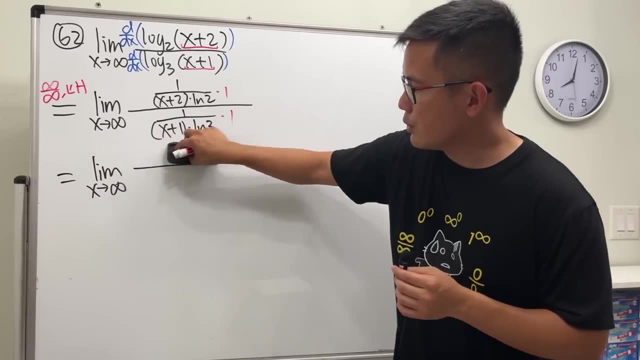 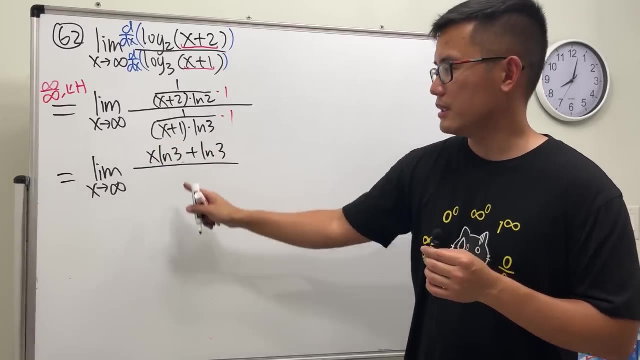 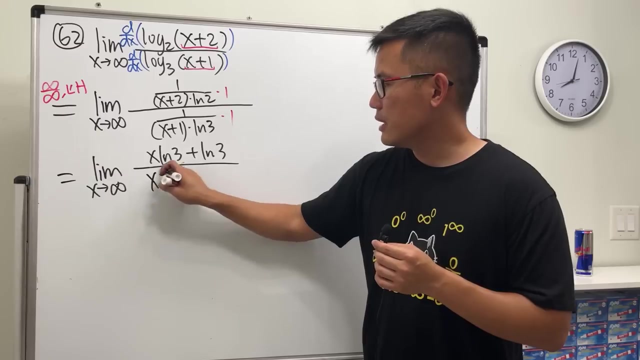 as x approaching infinity. and then we have x plus 1 times. let's distribute, you will see why, and let's see how do we write it. let's do this x times ln 3 plus ln 3, distribute, and ln 3 is the constant, it's the coefficient of x. and then this, right here, same thing, x. 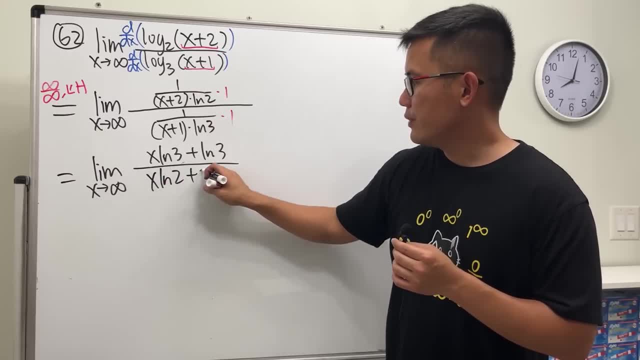 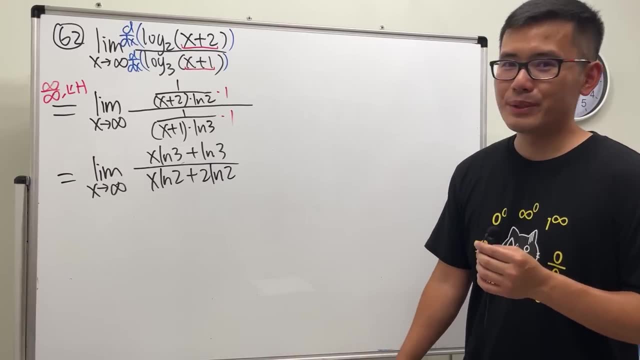 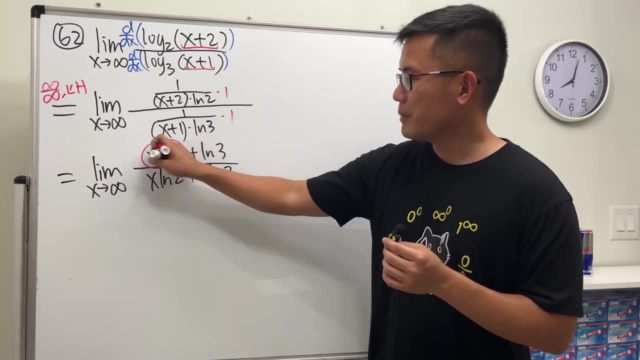 ln 2 plus 2 ln 2. but guess what? this is everybody's favorite derivative. this is everybody's favorite derivative. this is everybody's favorite limit question, calculus question. because x is approaching infinity, just care about the x to the first power, the dominating x, right yeah? 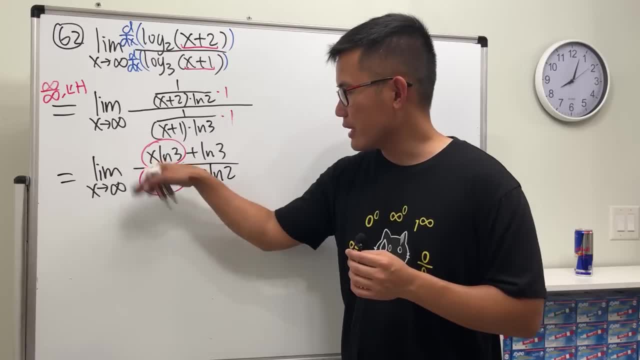 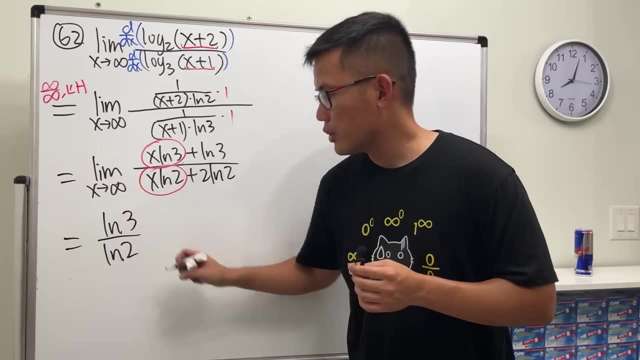 yeah, they have the same degrees in power, so they cancel. and then it's just ln 3 over ln 2, isn't it good? and now, icing on the cake, we can use the change of base formula and write this as ln 3 over ln 2. 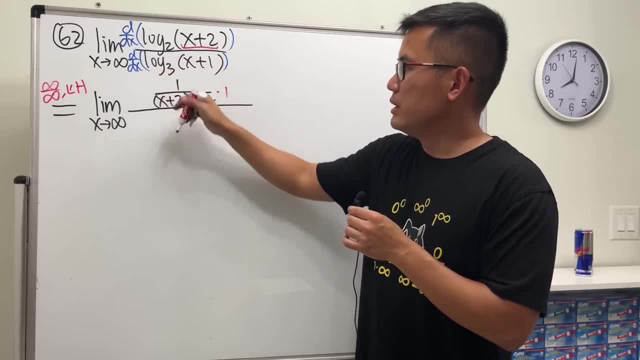 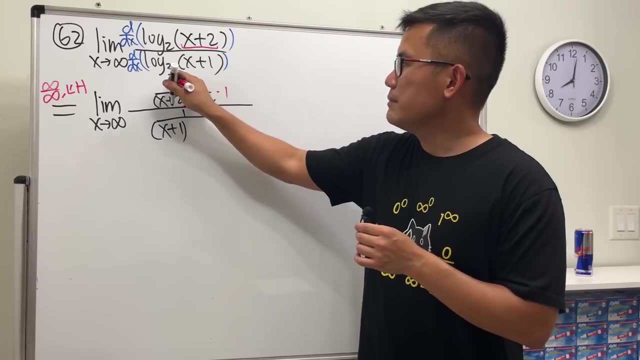 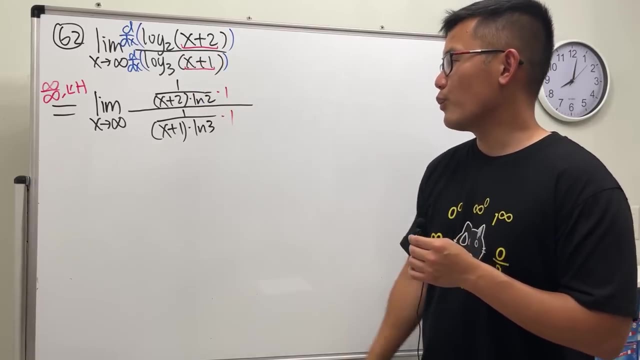 All right, let's practice this again. Derivative of log base 3 of x plus 1, you put this on the bottom first, so it's 1 over x plus 1.. Times ln3, okay, And then multiply by the derivative of this, which is also 1.. 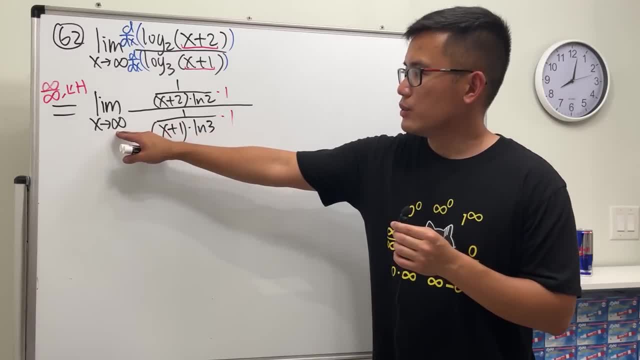 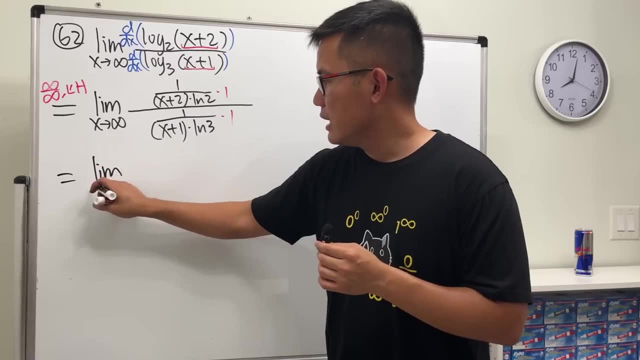 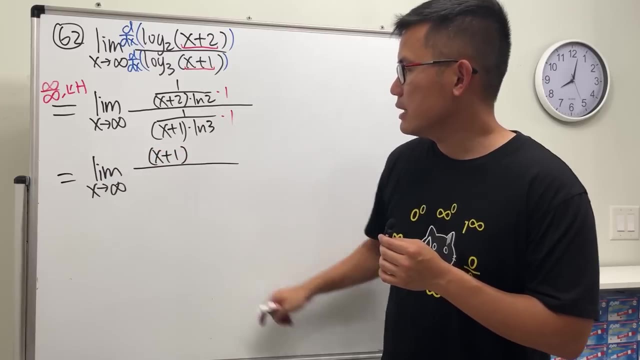 Cool. Now we want the x to be going to infinity, but let's just put this on the top. So, on O, we are looking at the limit as x approaching infinity, And then we have x plus 1 times. let's distribute, you'll see why. 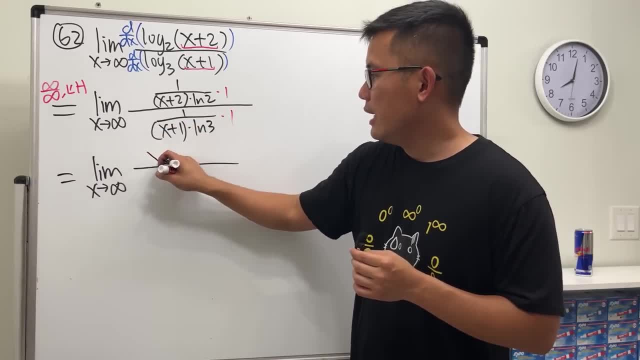 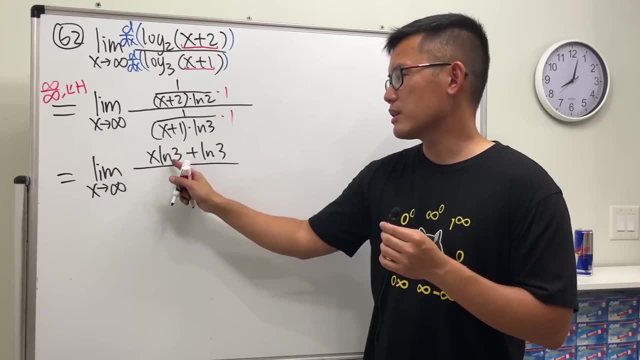 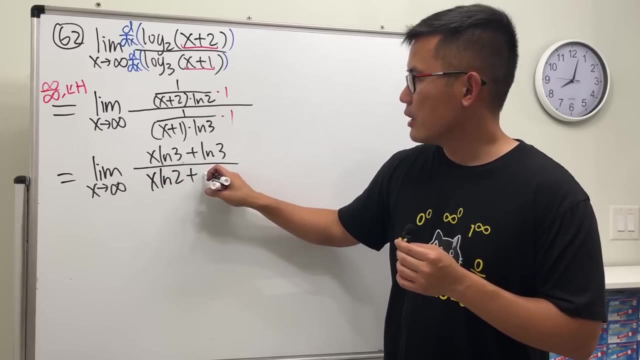 And let's see how do we write it. Let's do this: x times ln3 plus ln3.. Okay, distribute, And ln3 is the constant, it's the coefficient of x. And then this, right here, same thing: x ln2 plus 2 ln2.. 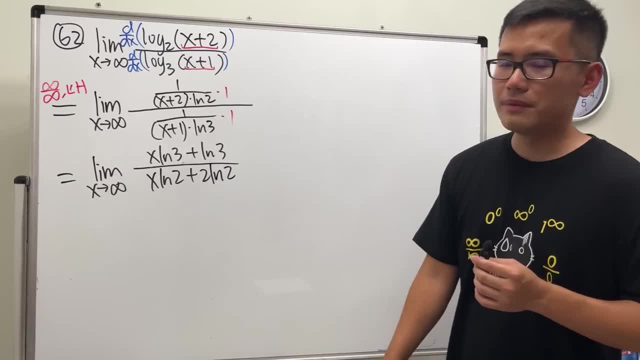 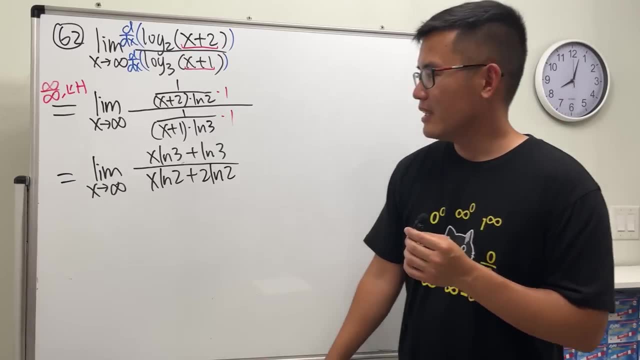 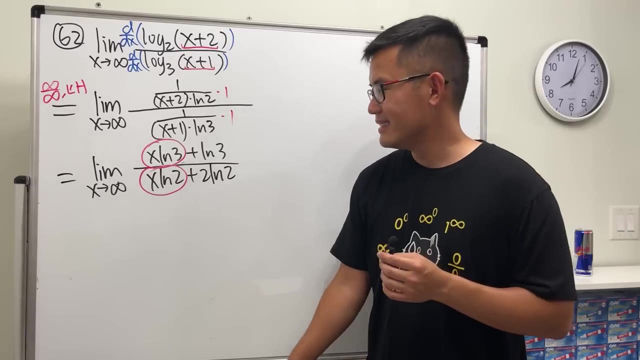 But guess what? This is everybody's favorite derivative. This is everybody's favorite limit equation, calculus equation, Because x is approaching infinity. Just care about the x to the first power, the dominating x, right? Yeah Yeah, They have the same degrees in power, so they cancel. 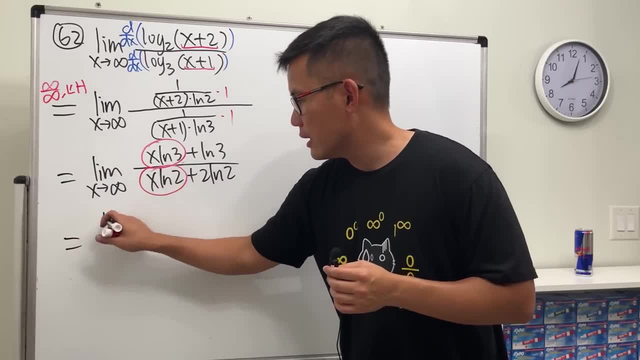 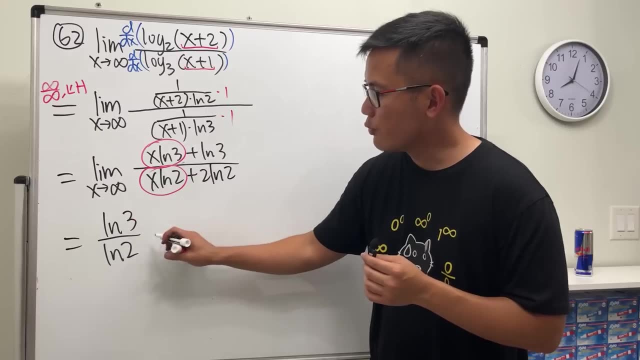 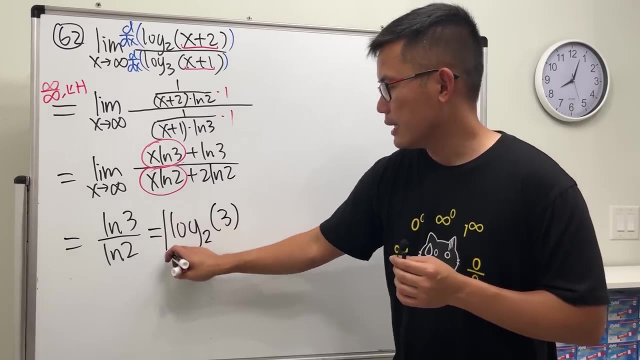 And then it's just ln3 over ln2,, isn't it Good? And now, icing on the cake, We can use the change of base formula and write this as log base 2 of 3.. Aha, Oh my goodness. 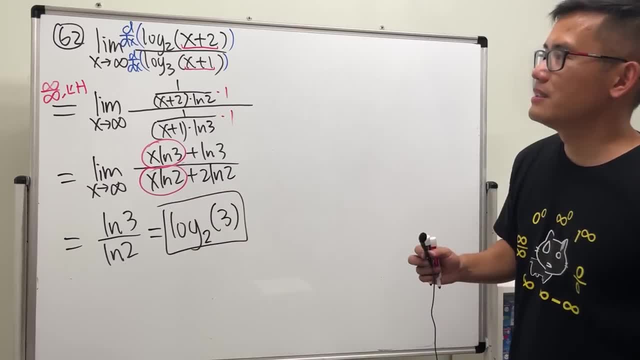 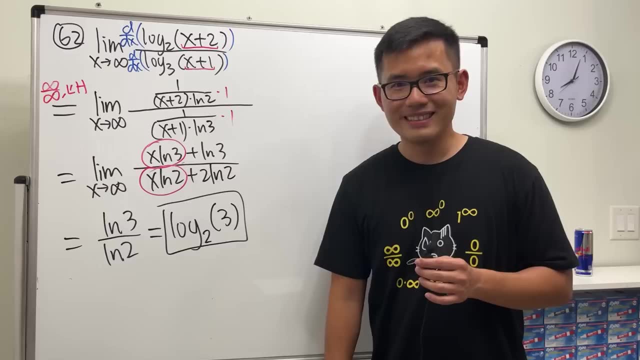 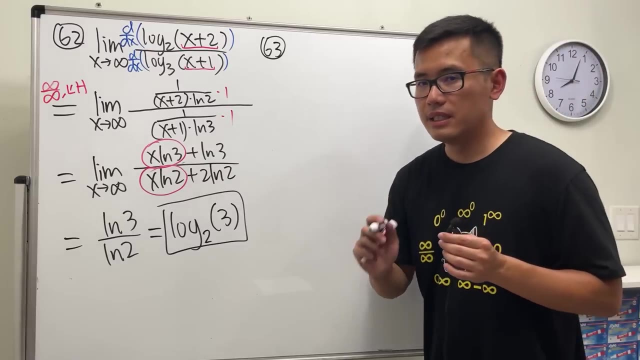 Log base 2 of 3.. Not kidding, This right here is the answer for that. So you see, infinity over infinity, we get like a irrational number. Yeah, Okay, Okay. Number 63.. One of the classic calculus questions. 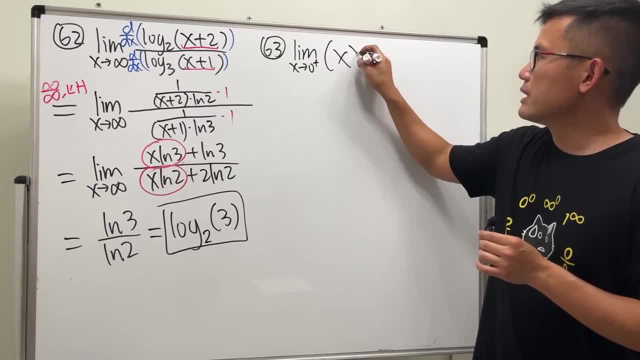 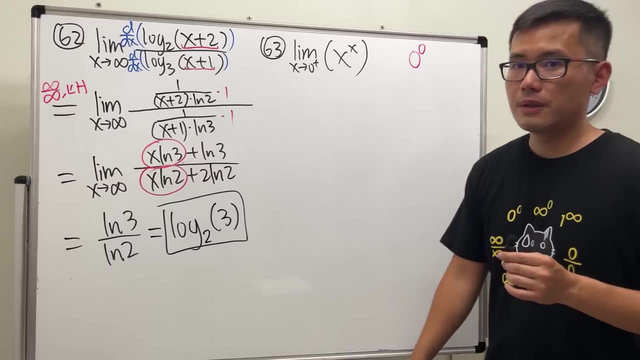 Limit as x approaching 0 plus x to the x power. Check this out: If we put 0 into here and here, we are getting 0 to the 3.. 0 to the 0 is power. Let me tell you, if you're just talking about computation, 0 to the 0.. 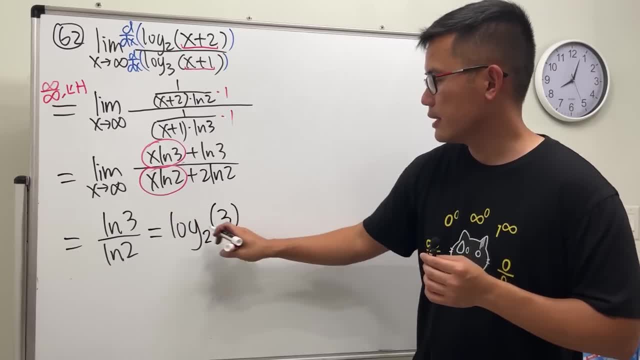 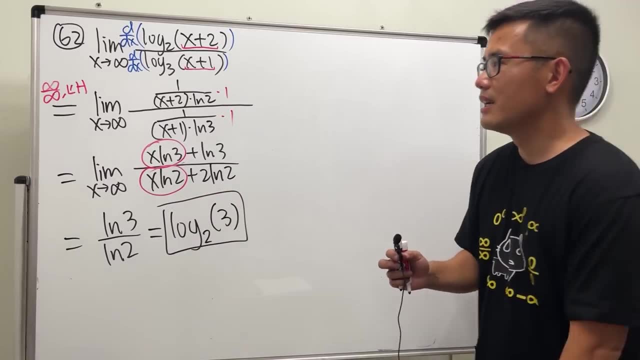 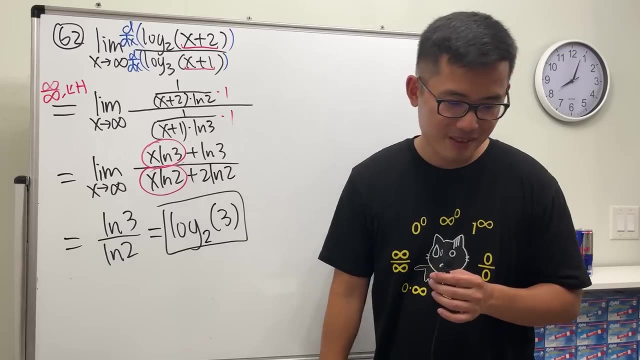 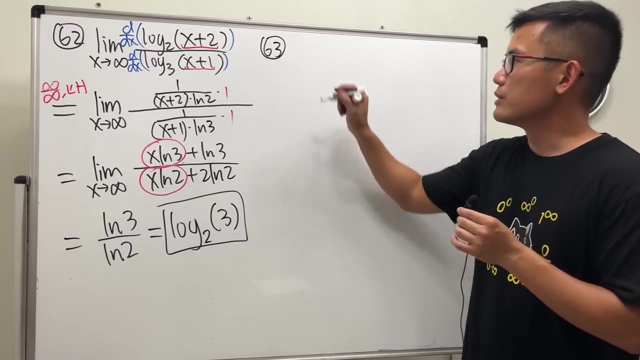 base two of three. oh, my goodness, log base two of three, not kidding, this right here is the answer for that. so you see, infinity over infinity, we get like, uh, irrational number, yeah, okay, number 63, one of the classic calculus question limit as x approaching zero plus. 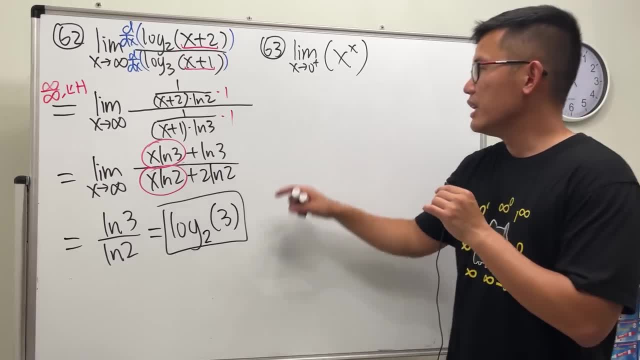 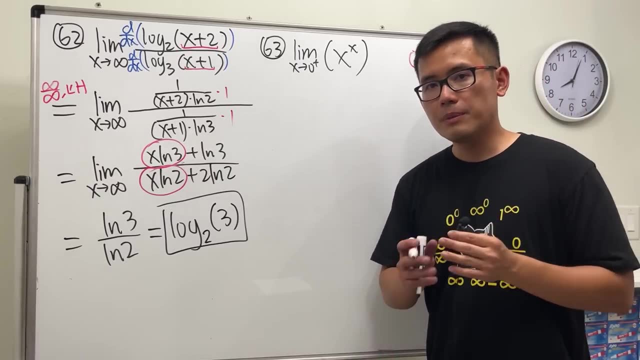 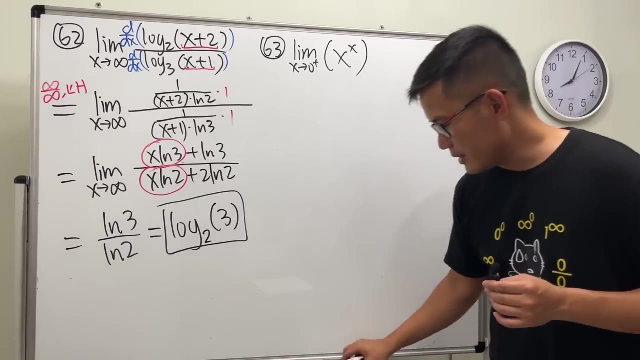 x to the x power. check this out: if we put zero into here and here, we are getting zero to the zero's power. let me tell you, if you're just talking about computation, zero to the zero, okay, i'm just going to do this like- more legitimately, i'll say, for limits. 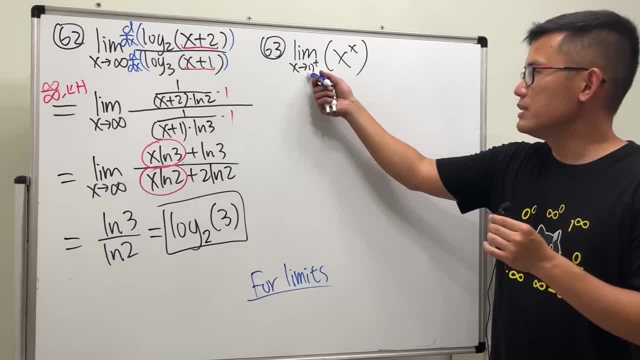 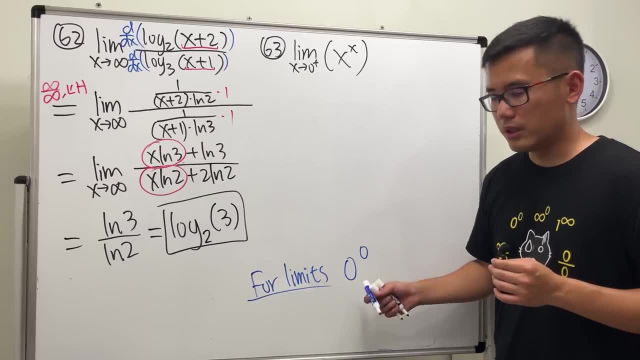 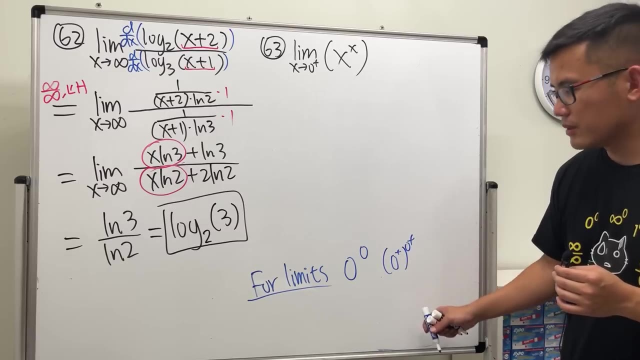 and again for limit means that the limit for meaning. i just put this number into here and here and just get the form of it. technically it's a zero plus to a zero plus right. but usually we just write zero to the zero, but again it's really zero plus to the zero plus right, like that okay. 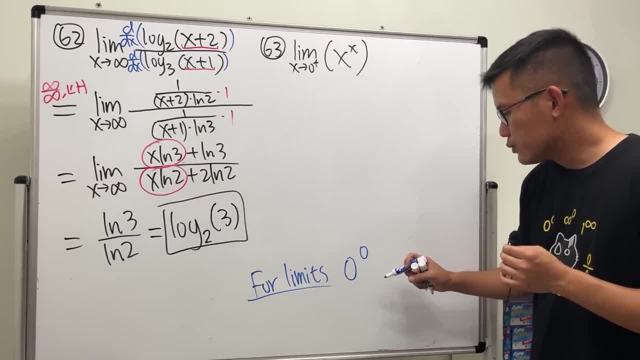 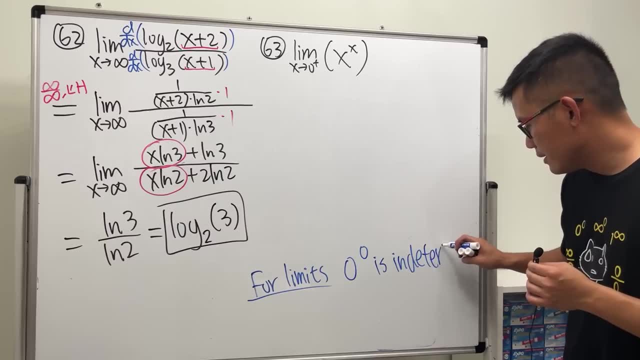 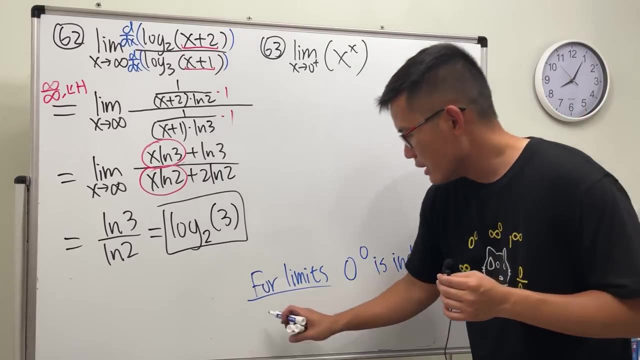 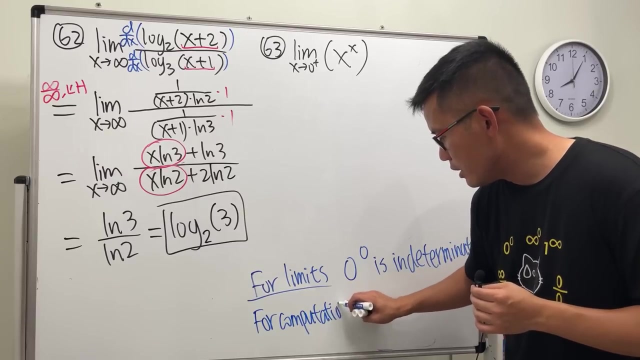 but anyway, when we have this limit form, this right here is in the in the terminate. okay, why? inside one here, it's right here, okay. but anyway, if today we're just doing computation- and by computations i mean that you know, when you have two to the third power, what do we do? 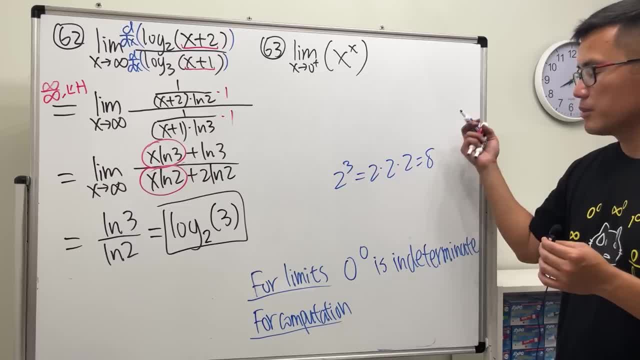 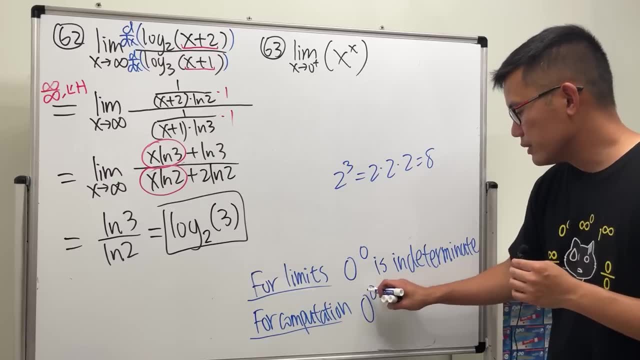 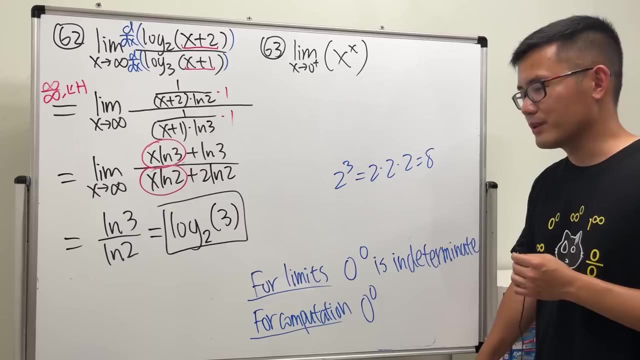 you just do two times, two times two, three times, that's computation. but anyway, when we're just talking about computation like no calculus with no limit involved, zero to the zero, this right here is the most debatable number or number of points or anything i don't know. a lot of people will say this right here is undefined. 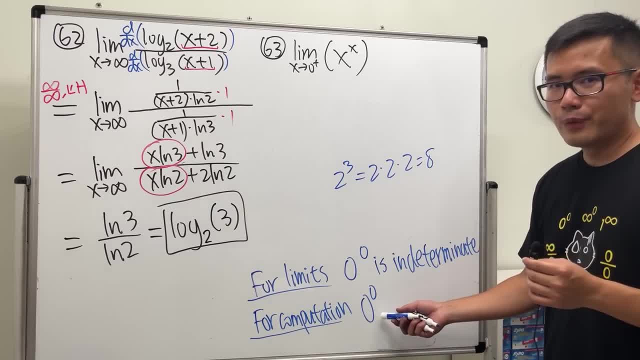 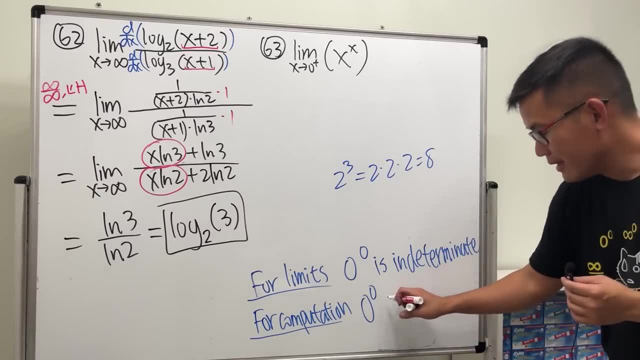 i used to say that, and a lot of people will also say this right here- should be equal to one. i would like to tell you, for computation, this right here- i think the best answer that i can tell you is that this right here has no agreement. i think this is the best answer that i can say. i know. 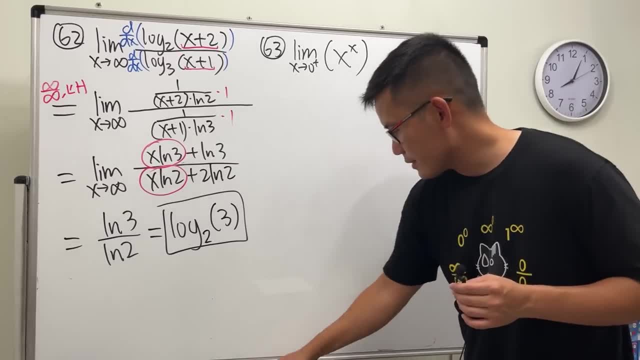 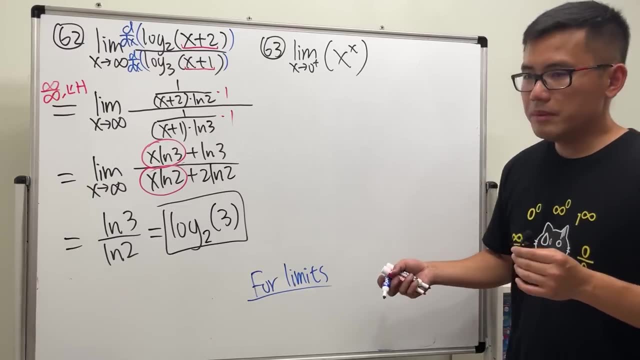 Okay, I'm just going to do this more legitimately. I'll say for limits. And again: for limit means that the limit for me- I just put this number into here and here and just get the form of it Technically, it's a 0 plus to a 0 plus, right. 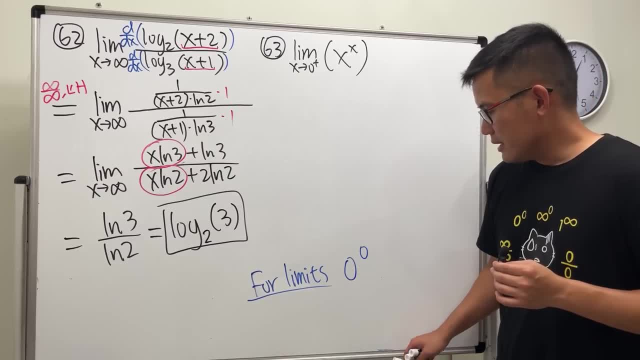 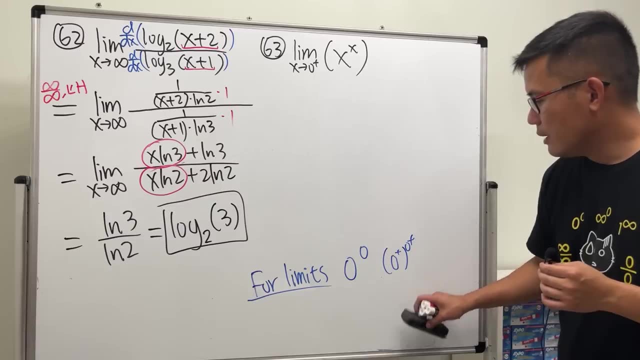 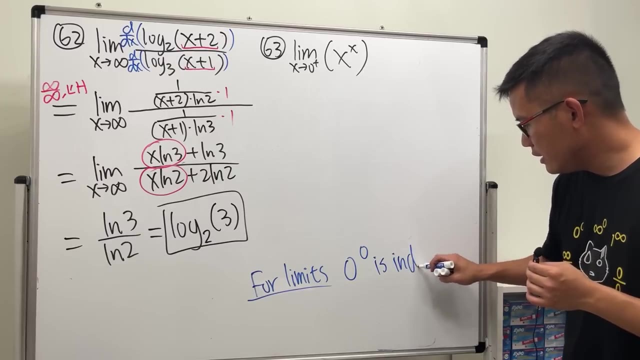 But usually we just write 0 to the 0. But again it's, It's really 0 plus to the 0, plus like that. Okay, But anyway, when we have this limit form, this right here is indeterminate. 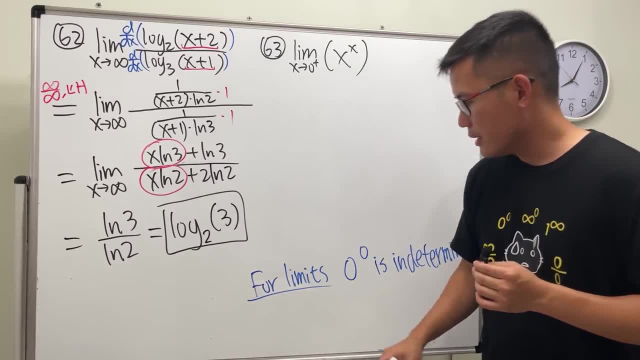 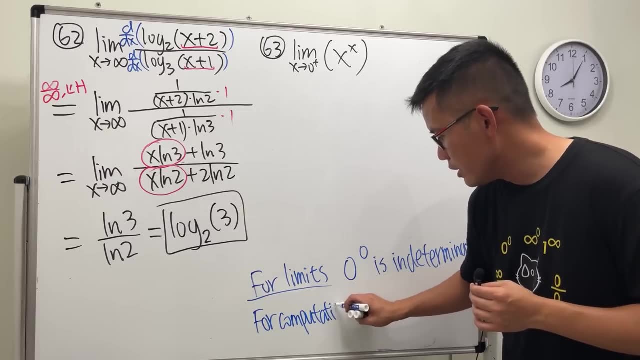 Okay, Why It's right here. It's right here, Okay. But anyway, if today we're just doing computation- And by computations I mean that you know, when you have 2 to the 3rd power, what do we do? 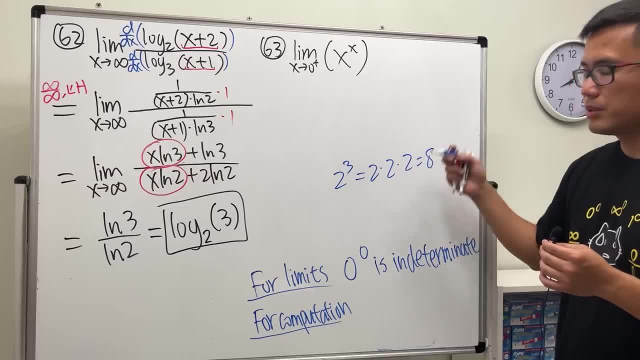 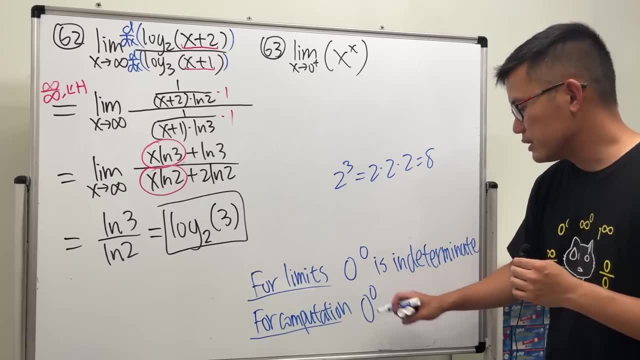 You just do 2 times, 2 times 2,, 3 times. That's computation. But anyway, when we're just talking about computation like no calculus with no limits involved, 0 to the 0, this right here is the most debatable number or anything. 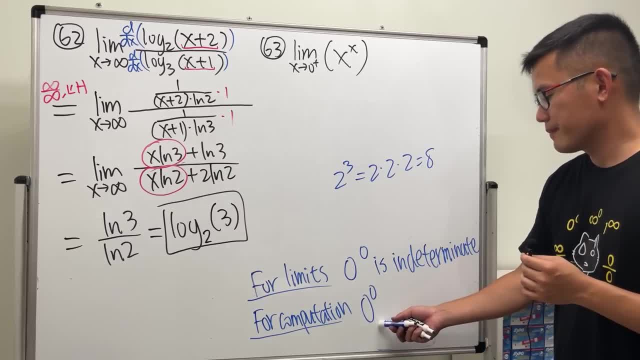 I don't know. A lot of people will say this right here is undefined. I used to say that, And a lot of people will also say this right here should be equal to 1.. I would like to tell you, for computation, this right here. 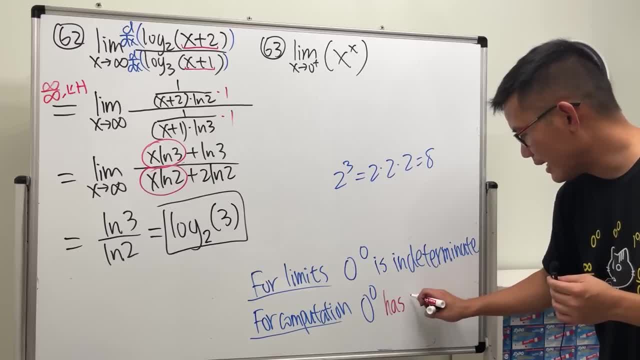 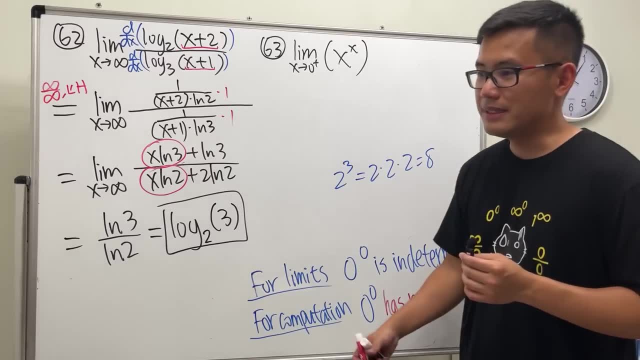 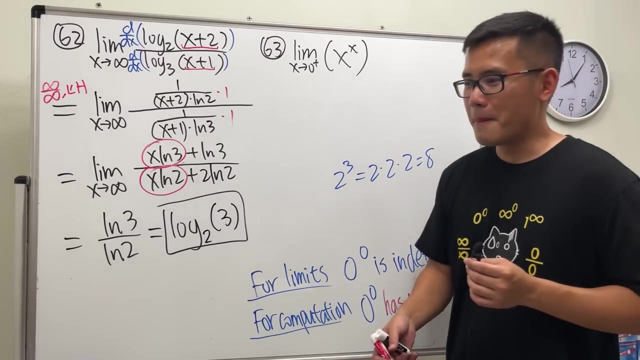 I think the best answer that I can tell you is that this right here has no agreement. I think this is the best answer that I can say. I think people will agree that there's no agreement on this. If you really want to say, this is 1, then you can make a Facebook post for like a YouTube video. 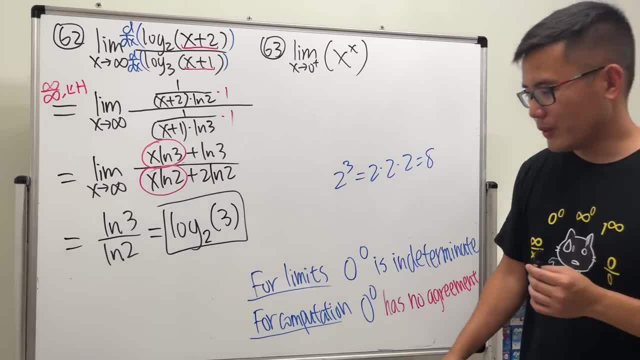 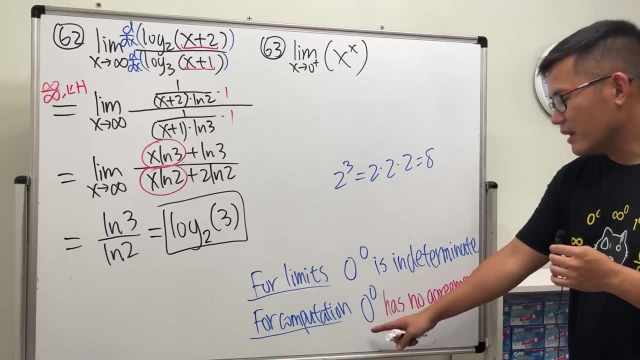 Or like a Twitter And then you can see how many people will like debate and all that. If you say this is undefined, you know same thing will happen. But if you say this right here has no agreement, hopefully you guys leave me alone. 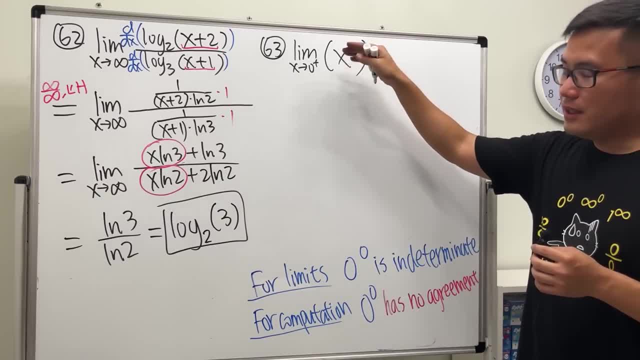 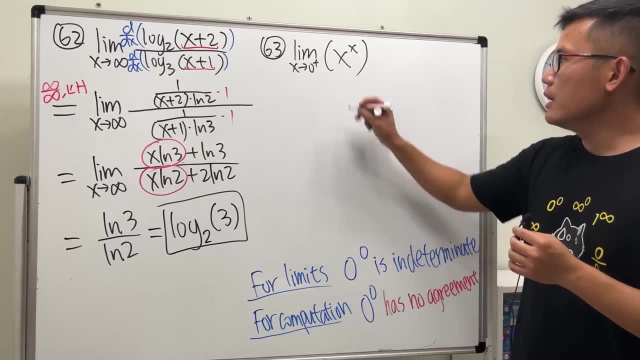 But anyway, this right here is 0 to the 0, but we're doing limits, So it's indeterminate, meaning we have to do more work. This is how. Okay, We like base x. we like to have base e. this is the fast way to do it. 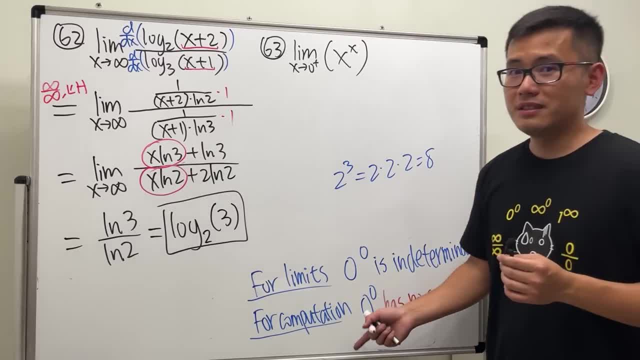 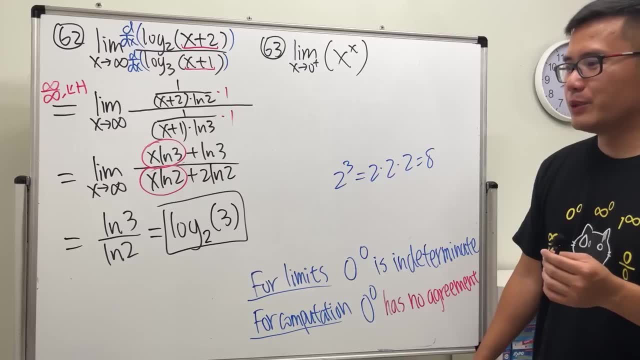 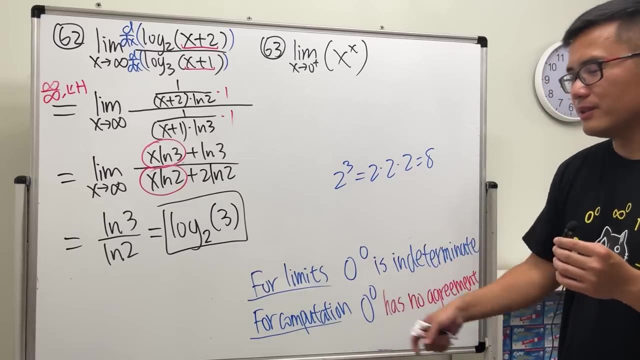 i think people will agree that there's no agreement on this. if you really want to say this is one, then you can make a facebook post for like a youtube video or like a twitter, and then you can see how many people will like debate and all that. if you say this is undefined, you know. 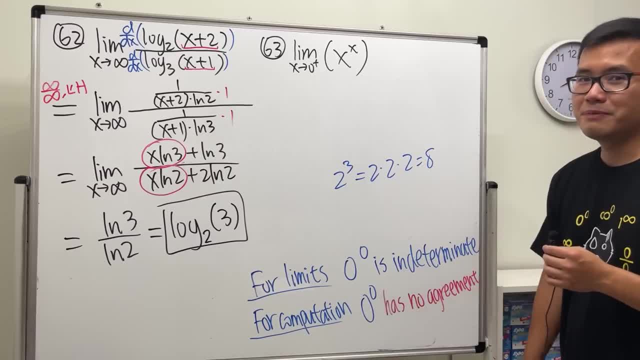 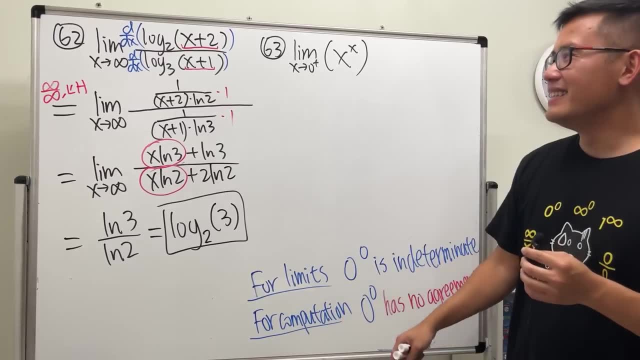 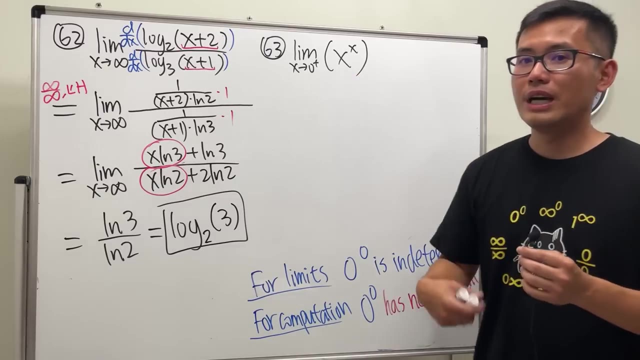 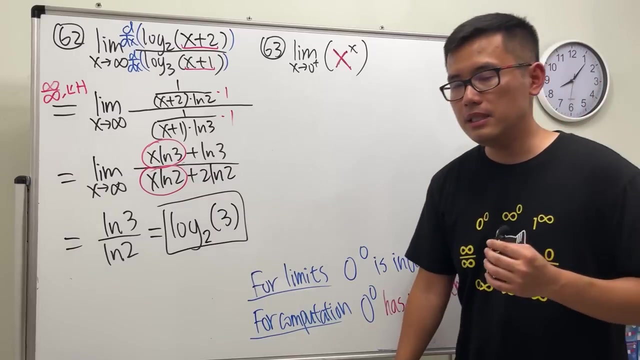 sensing will happen. but if you say this right here has no agreement, hopefully you guys leave me alone. but anyway, this right here is your open. this is right here: zero to zero. but we're doing limits, so it's indeterminate, meaning we have to do more work. this is how we don't like base x, we like to have base e. 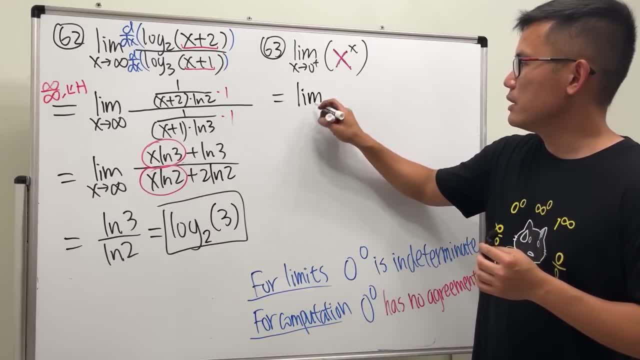 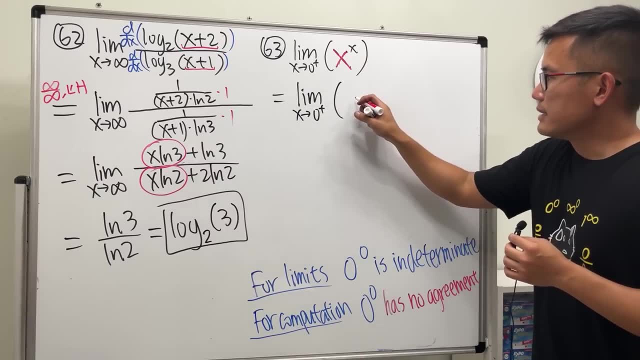 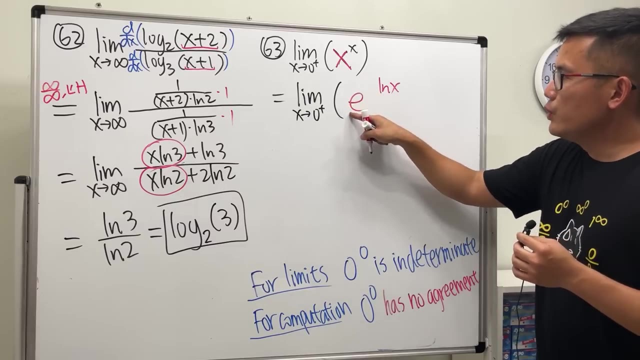 this is the fast way to do it: change the base to e, and we can achieve that by doing this: write x as e to the ln x power, because e and ln cancel, still get the x back, and then, you see, we're going to have to raise this to the x power, right? so, perhaps because this is the first time we're- 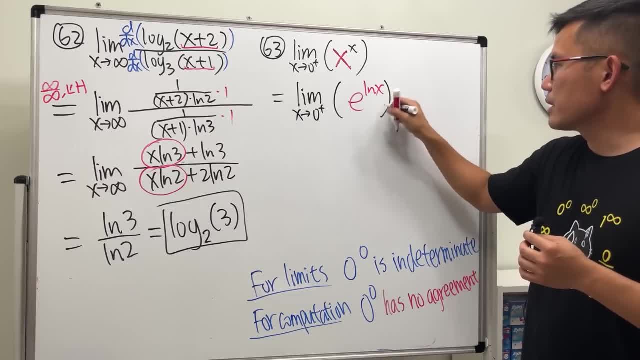 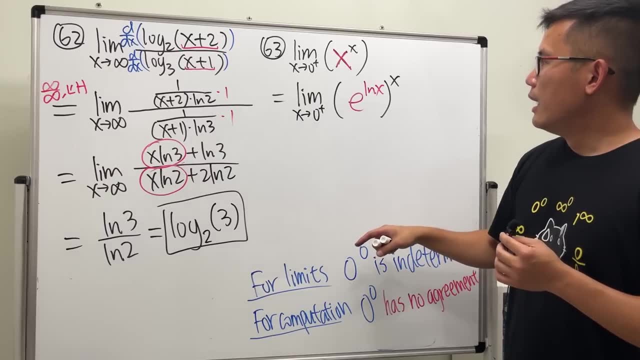 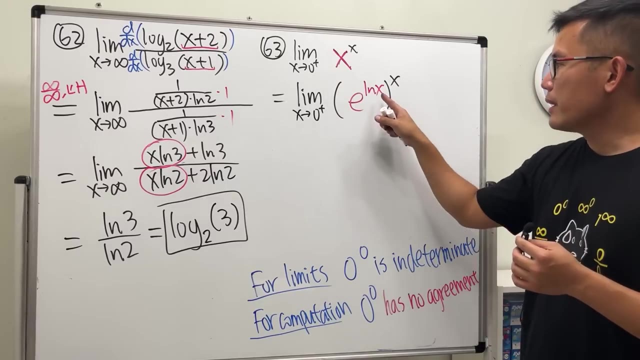 doing it. so i will show you guys a step by step, like this. i'm not going to skip anything, right? so this is x raised to the x power, okay. and then you might be wondering, you know the parentheses wise, and says: just don't worry too much about it. yeah, i think this might be better, okay, anyway. 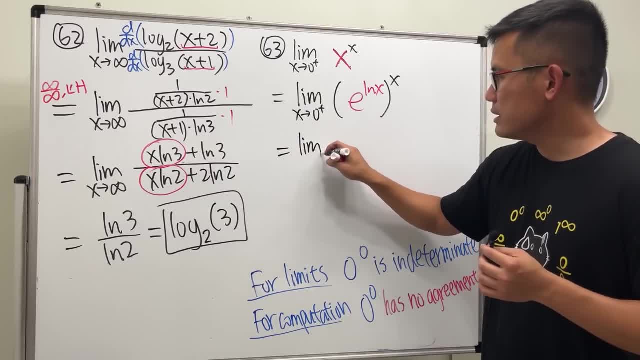 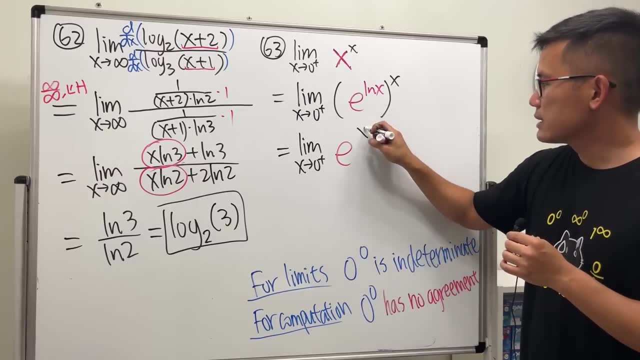 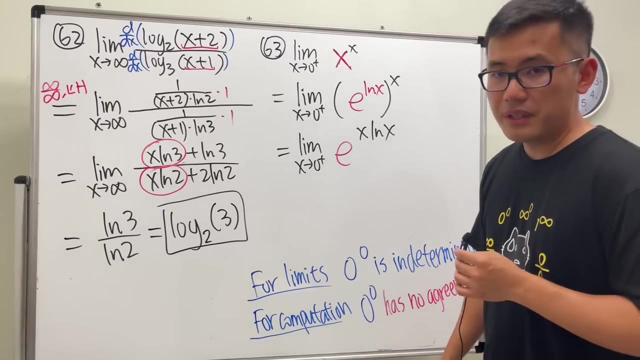 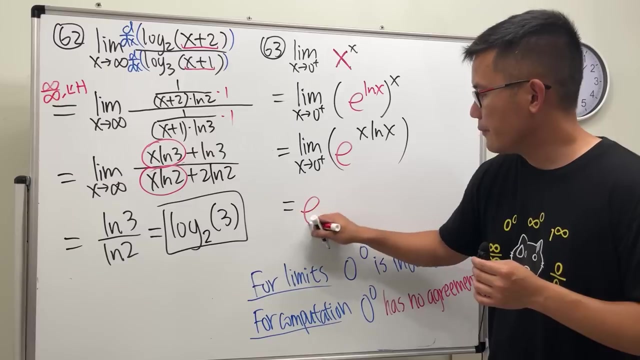 now i'm just going to write this as the limit as x approaching 0, plus we can multiply the powers and then we get e to the x times ln x power. does this look familiar? yes, it does. number 58, yes, but the way that you should take care of this is the following: this is e and 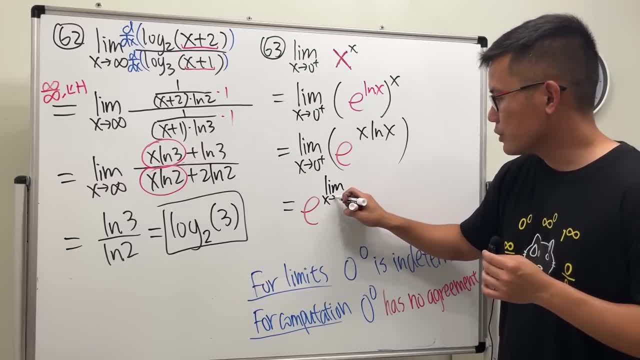 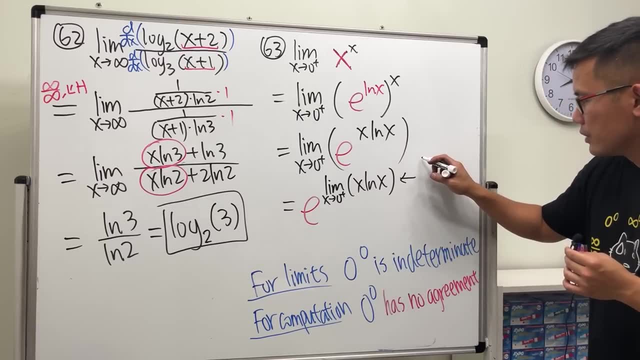 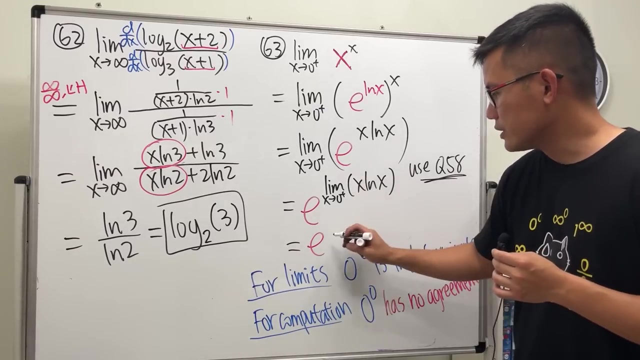 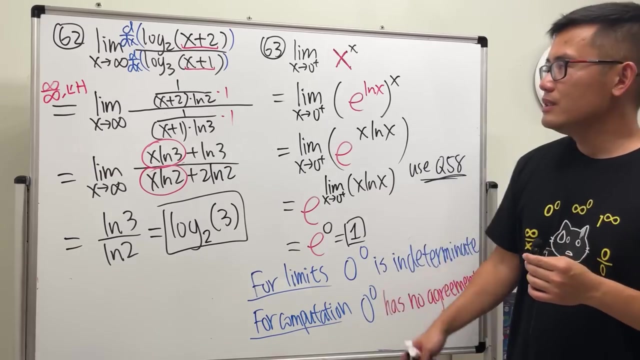 then you do the limit of that, which is the limit as x approaching 0 plus, and then just focus on x. as you say: um, use question 58, right? so in fact we get e, and earlier we saw that this is equal to 0. so, on all, we get one done. and of course, if you are doing this on the test, do not just say: look at 50. 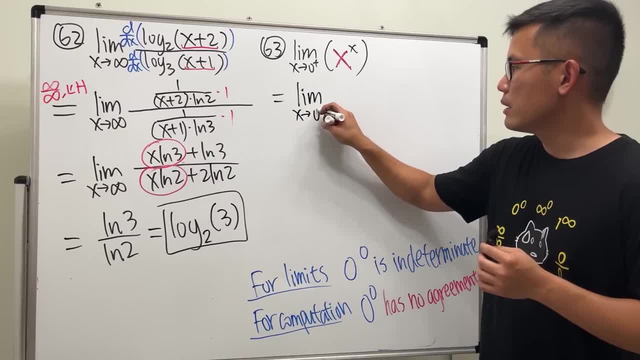 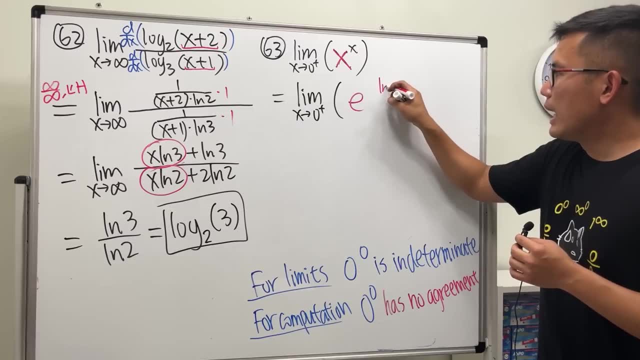 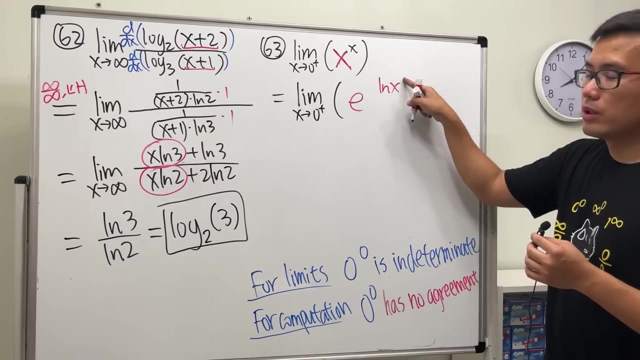 Change the base to e, And we can achieve that by doing this: Write x as e to the ln x power, because e and ln cancel still get the x back, And then, you see, we will have to raise this to the x power, right. 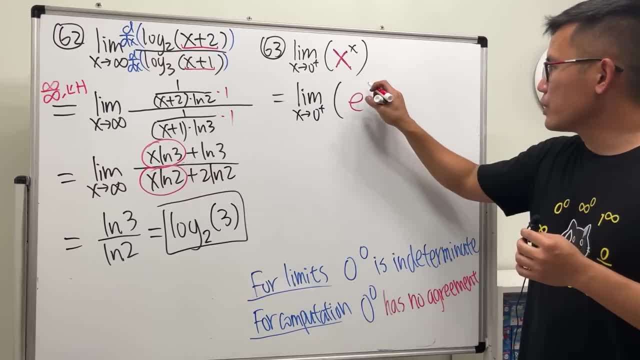 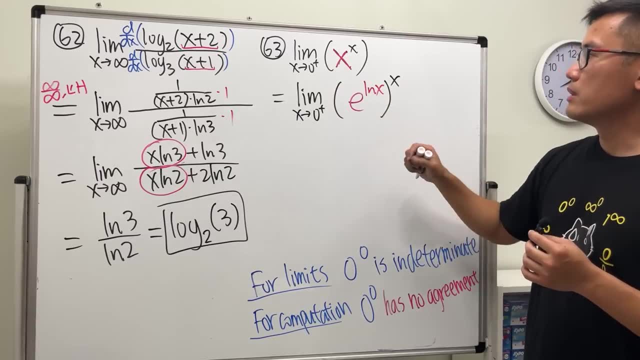 So perhaps because this is the first time we're doing it, So I will show you guys a step by step, like this. I'm not sure I'm not going to skip anything, right? So this is x raised to the x power. okay, 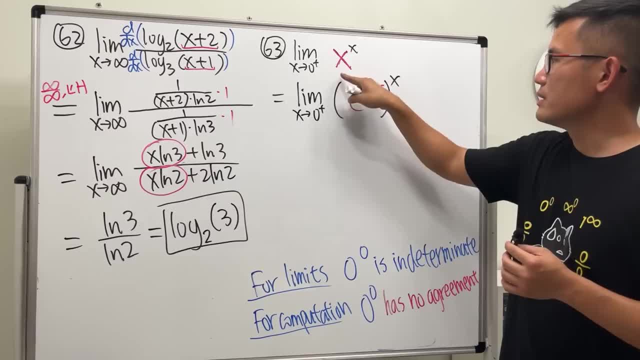 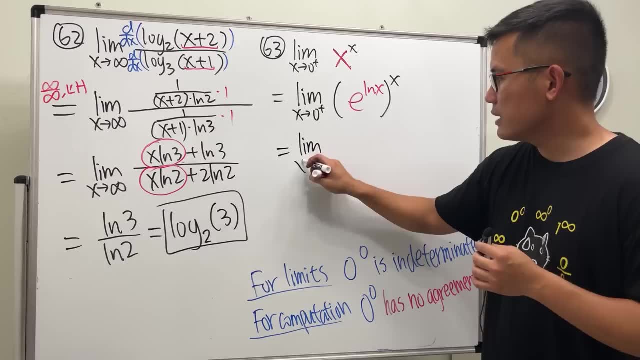 And then you might be wondering- you know the parentheses- why this is. just don't worry too much about it. Yeah, I think this might be better, okay, Anyway, now I'm just going to write this as the limit as x approaching 0 plus, we can. 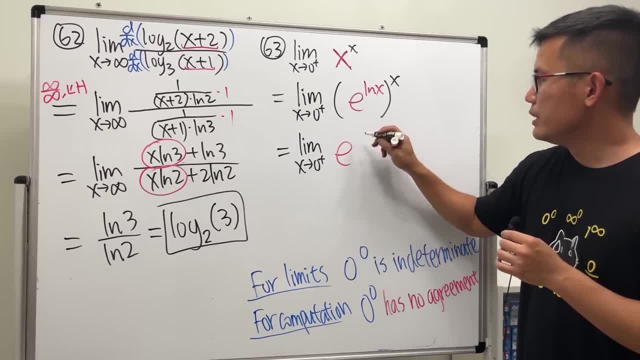 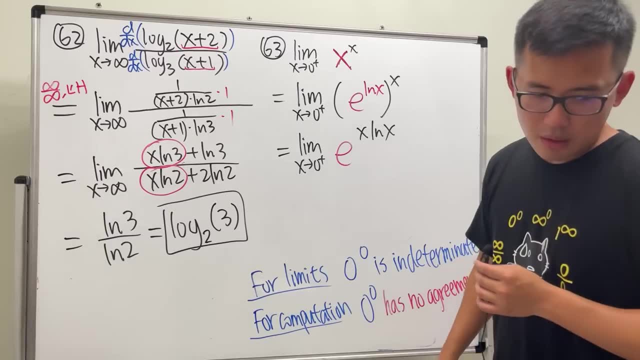 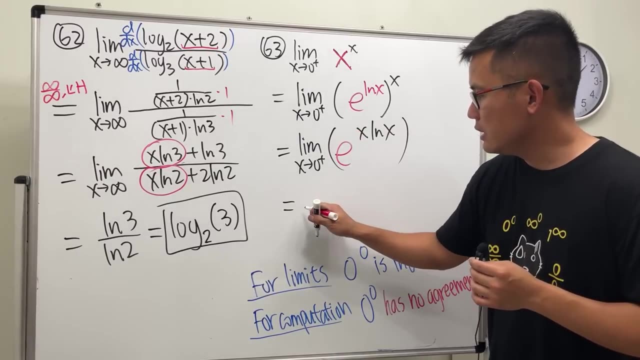 multiply the powers and then we get e to the x times ln x power. Does this look familiar? Yes, it does. Number 58. Yes, But the way that you should take care of this is the following: This is e, and then you do the limit of that, which is the limit as x approaching 0 plus. 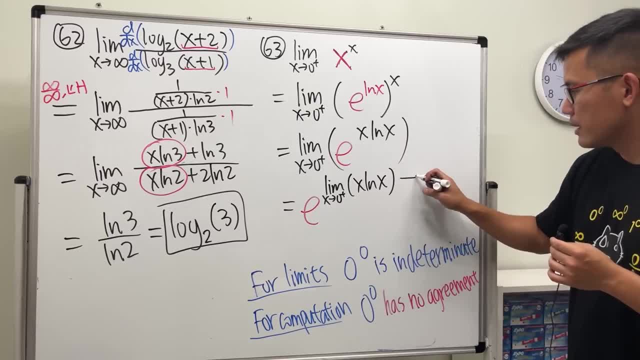 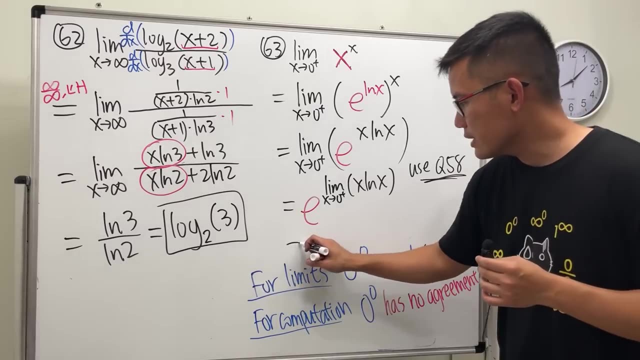 and then just focus on x, ln, x, But I should say use equation 58.. All right, So in fact we get e, and earlier we saw that this is equal to 0, so all in all we get 1.. 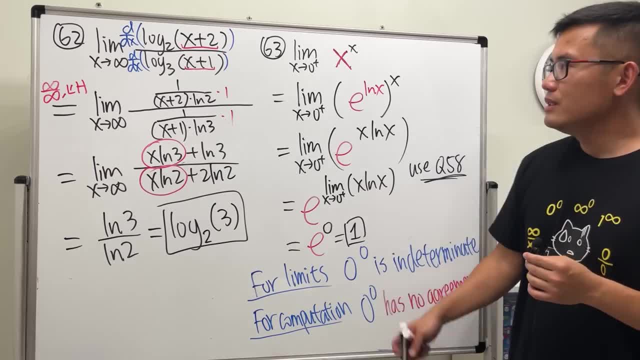 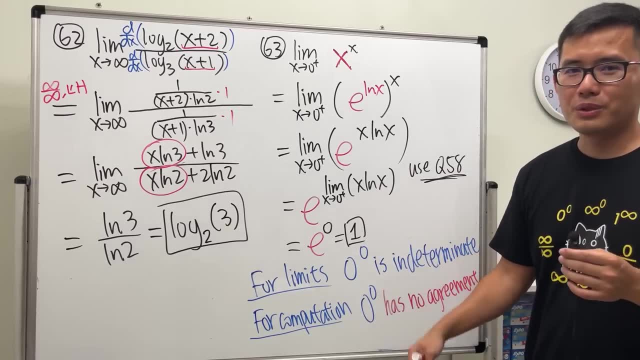 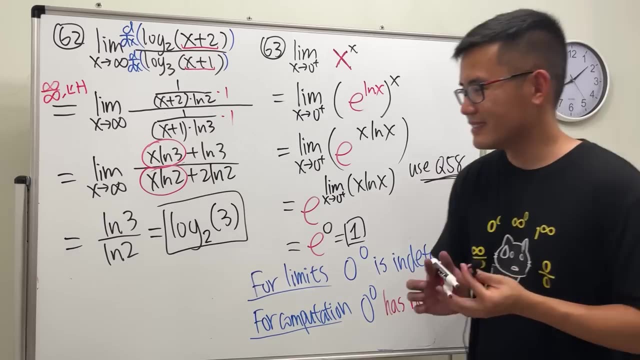 Done. And, of course, if you are doing this on a test, do not just say look at question 58. Nobody will know what you're talking about. Just redo everything from question 58 on your test so that people will be happy. 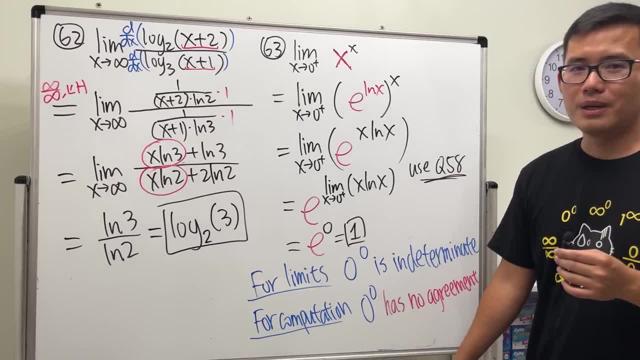 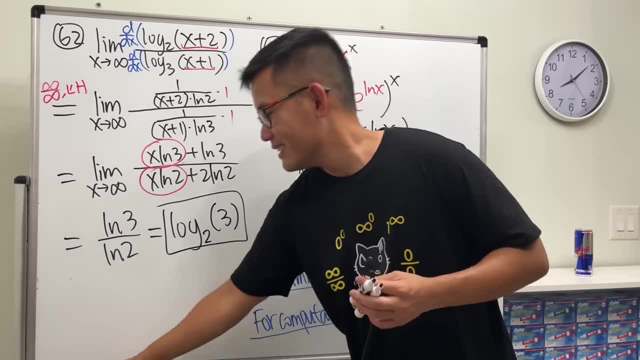 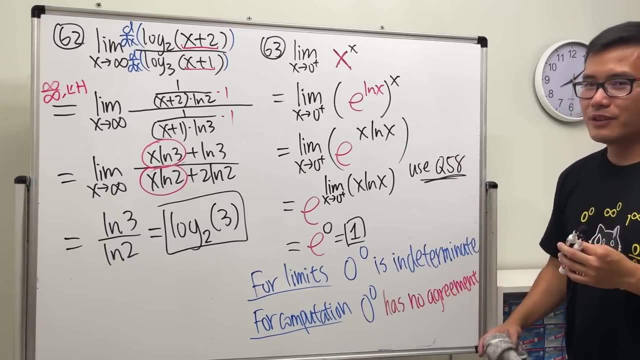 look at question 58. nobody will know what you're talking about. just redo everything from question 58 on your test so that people will be happy. okay, if my students, if you go from here to here and say, use question 58, i will give you focus. no, i will not give you full credit. 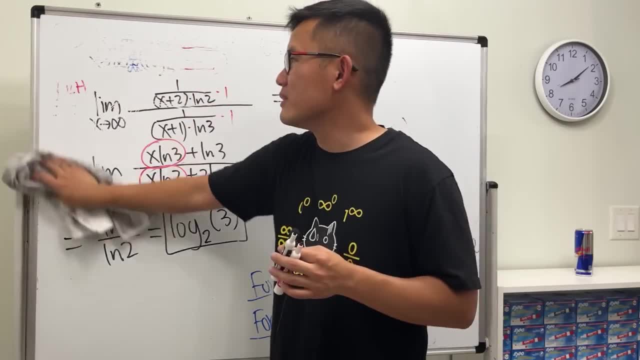 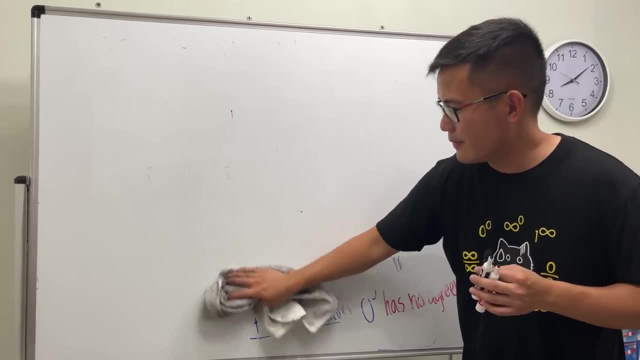 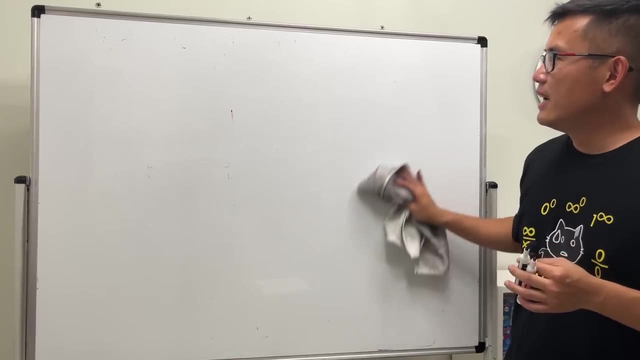 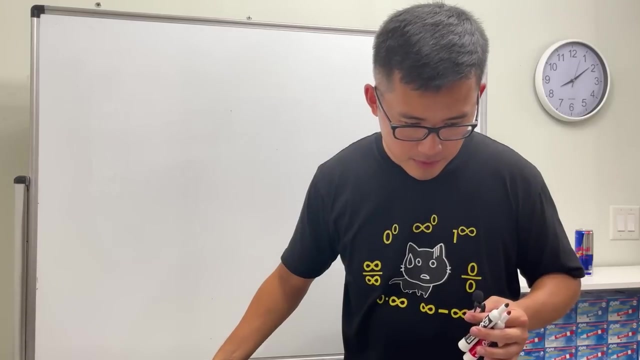 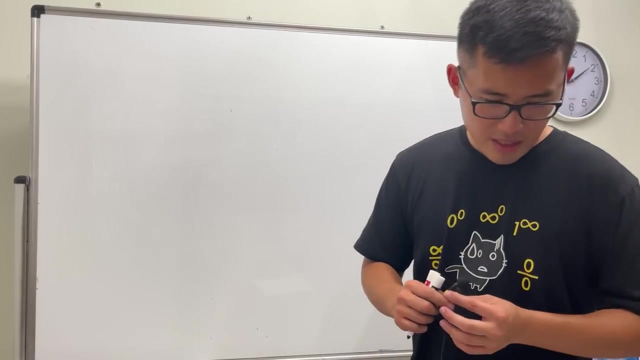 maybe i should, because i know that way you are watching my video. i don't know, but the deal is that will not ask you guys that question. this is too easy, or something more difficult. all right, all right. number 64: wow, that's eight square. 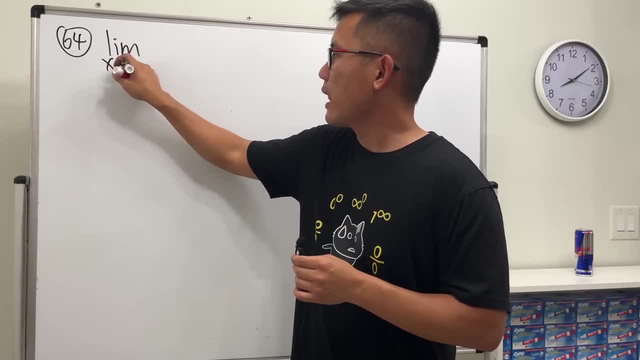 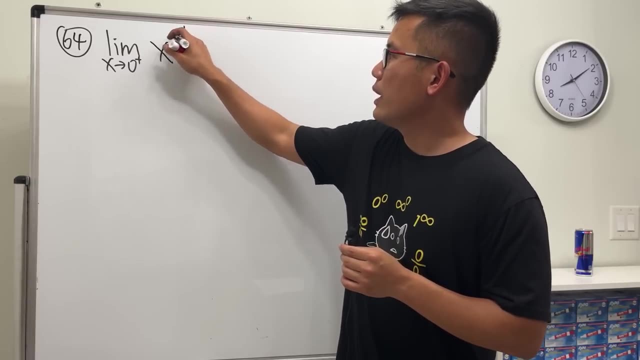 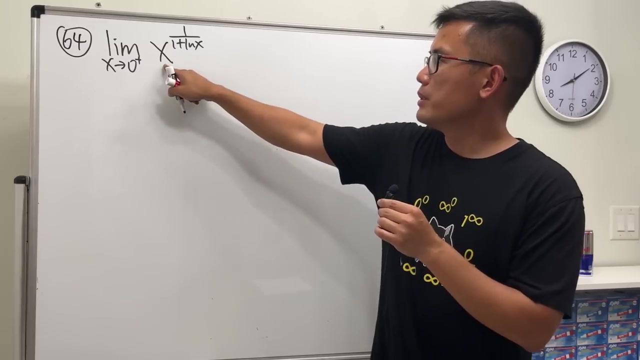 So limit is x approaching 0 plus, and here we have x to the 1 over 1 plus ln x power. And check this out: When we have 0 plus here, put it here: base is 0, and let's do this in our head. 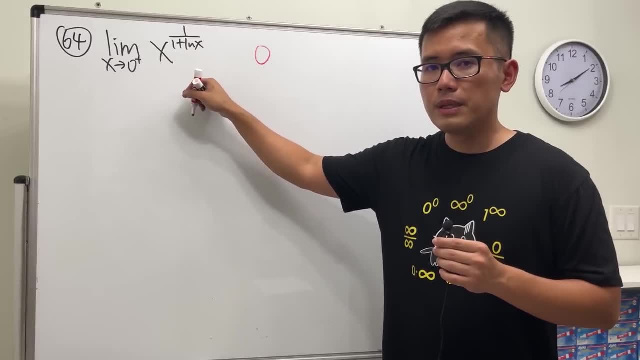 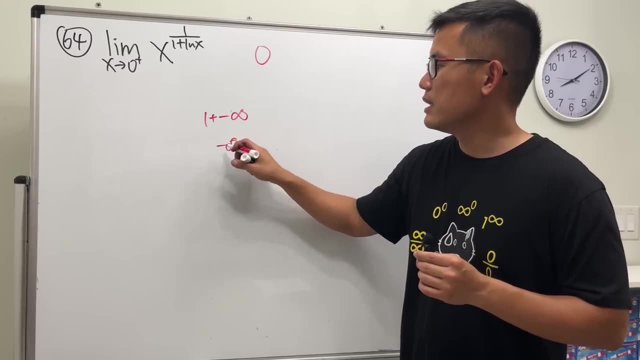 0 plus into ln. ln 0 plus is negative infinity. And then we have the 1, right: 1 plus negative infinity is just negative infinity, yeah, And then it's 1 over 1 over infinity is 0.. 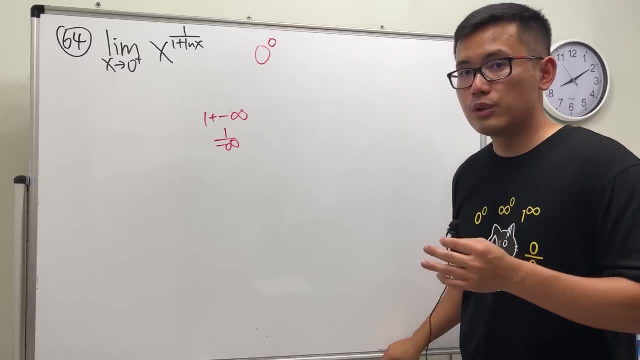 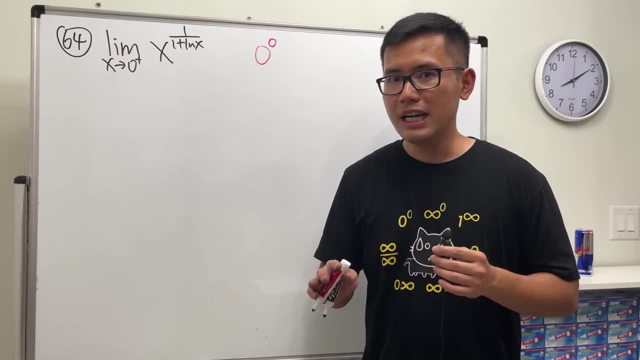 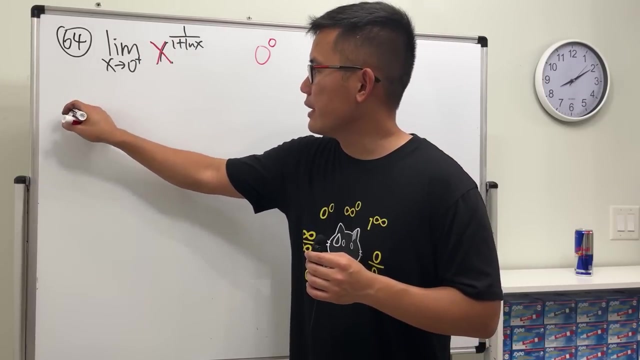 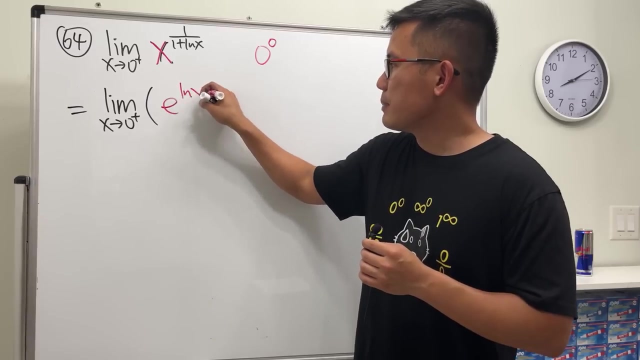 So this is actually a 0 to the 0 indeterminate form. Let's see if the answer is 1 or not. Do the same thing that we did earlier: Rewrite the x as e to the ln x. So this right here is the limit as x approaching 0 plus e to the ln x power. 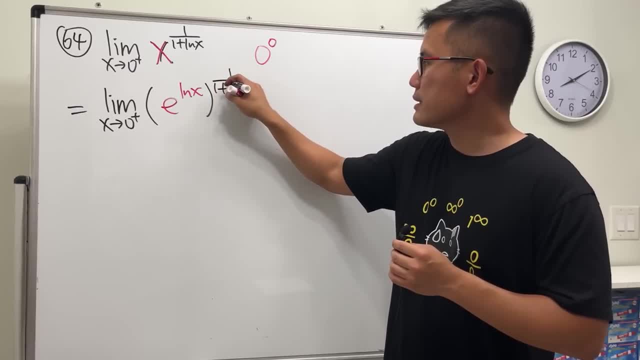 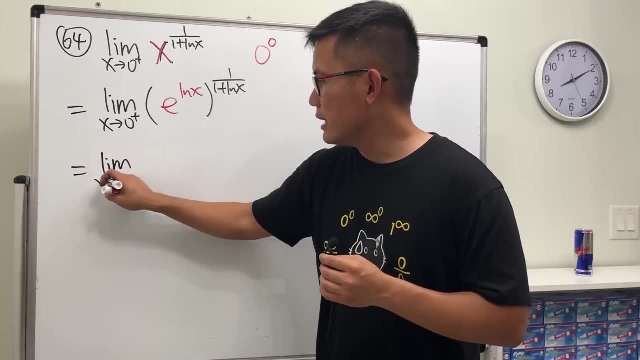 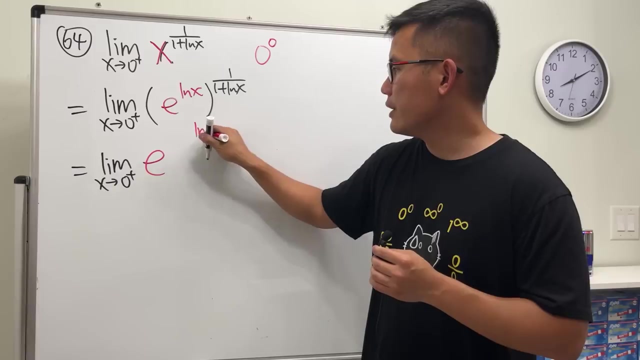 And then Then raise to the 1 over 1 plus ln x power. Now multiply the powers, So we are getting limit as x approaching 0 plus, and then we have just do it like this: e and then ln x over 1 plus ln x power. 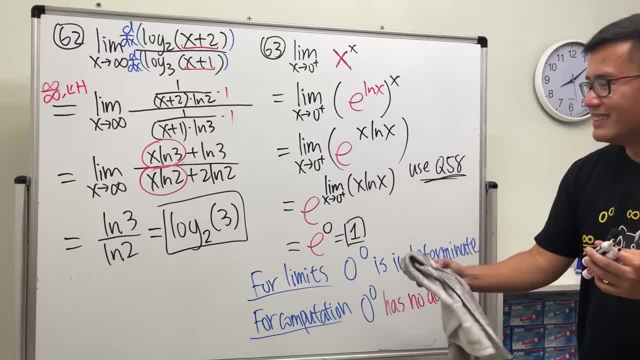 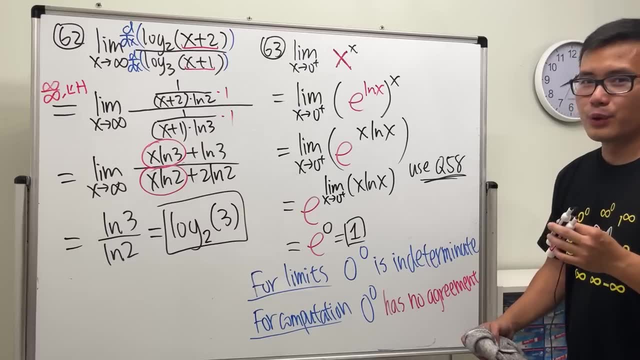 Okay, Okay. So, students, if you go from here to here and say use question 58, I will give you full credit. No, I will not give you full credit. Maybe I should, because I know that way you are watching my video. 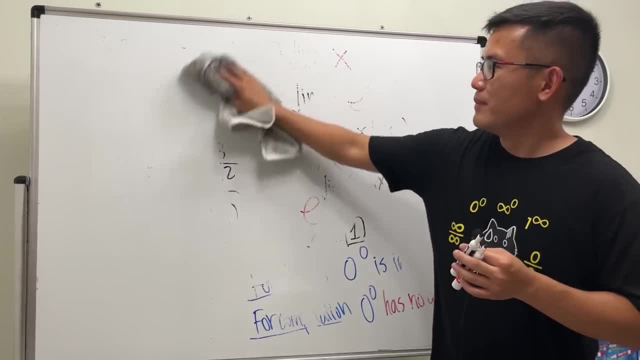 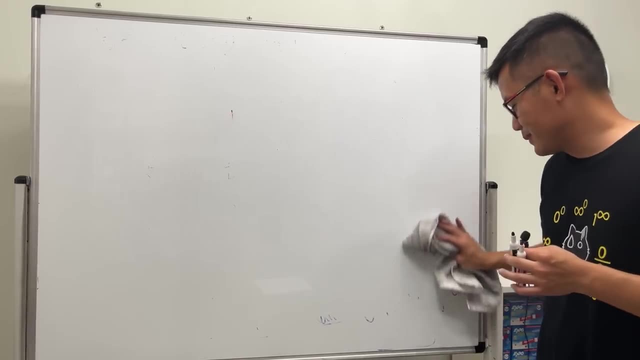 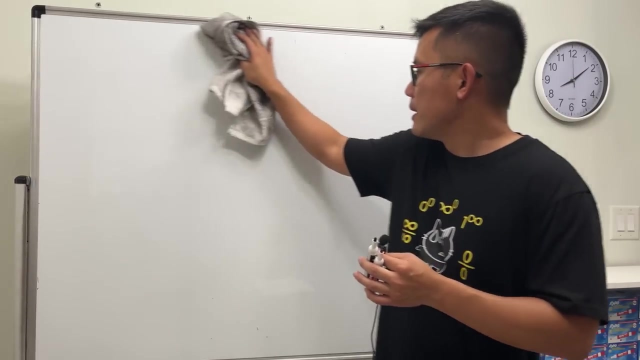 I don't know, But the deal is that I will not ask you guys that question. It's too easy. I'll ask something more difficult. Alright, All right, Alright, Number 64.. Oh, that's 8 square. So limit is x approaching 0 plus. 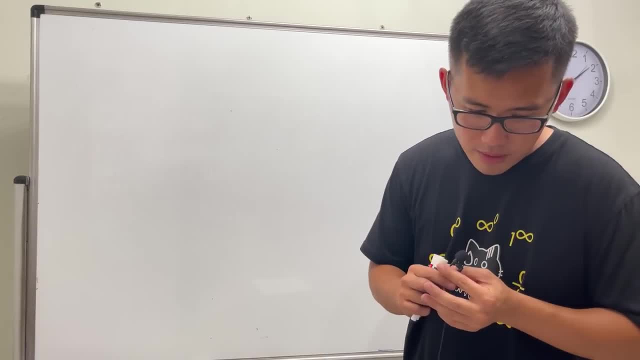 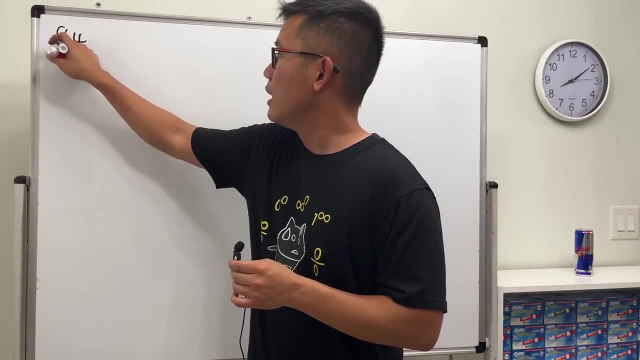 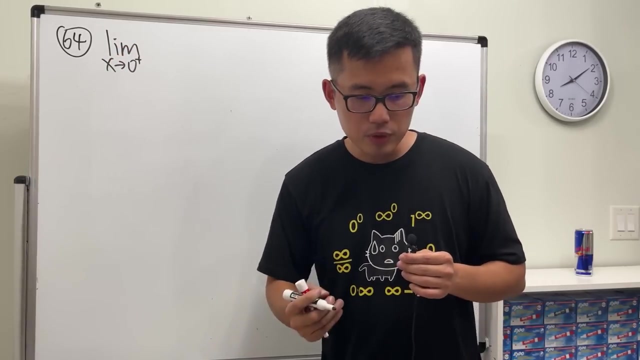 And here we have x to the 1 over 1 plus. So the 8 is 8.. Alright, Let's put in 4.. The limit is x to the 1 over 1 plus, And here we have x to the 1 over 1 plus. 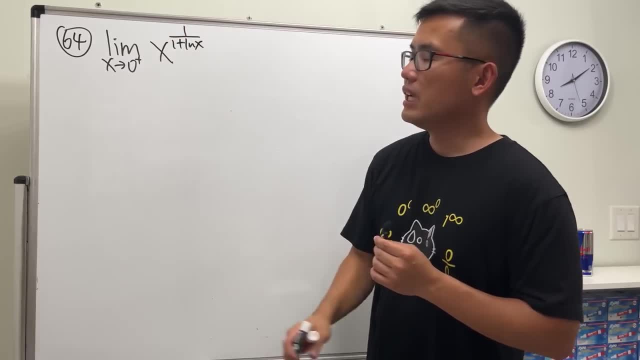 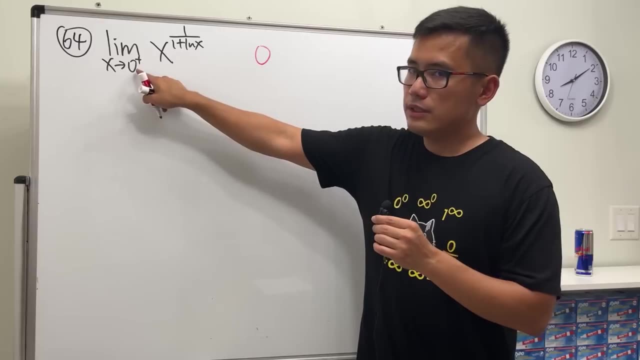 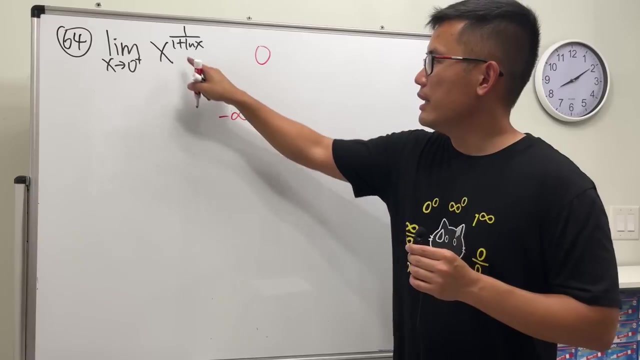 to the 1 over 1 plus ln x power and check this out. when we have 0 plus here, put it here: base is 0 and let's do this in our head: 0 plus into ln, ln, 0 plus is negative infinity, and then we have the 1. 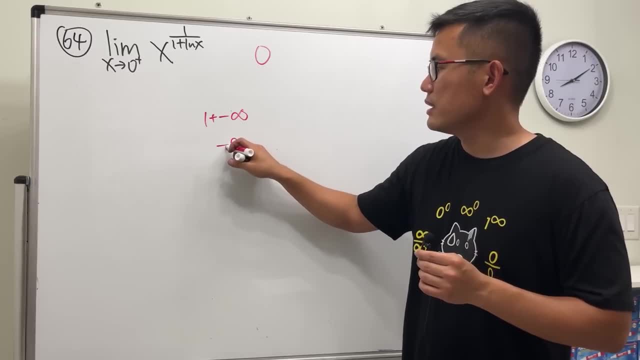 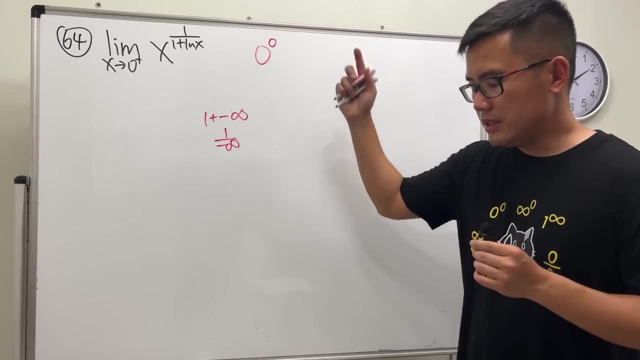 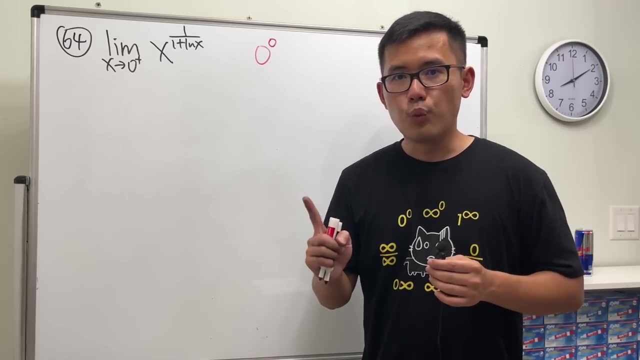 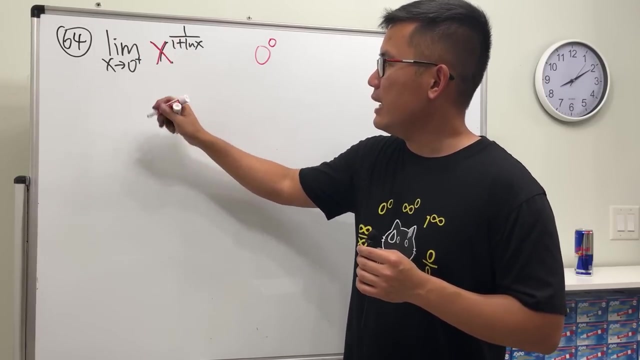 right. 1 plus 1 plus negative infinity is just negative infinity, yeah, and it's 1 over. 1 over infinity is 0, so this is actually a 0 over. this is actually a 0 to the 0 in determinant form. let's see if the answer is 1 or not. do the same thing that we did earlier: rewrite the x as e to. 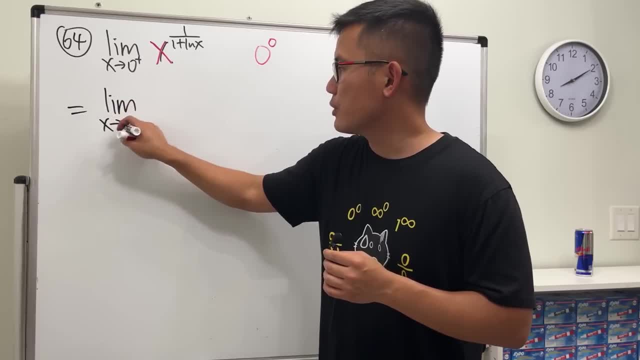 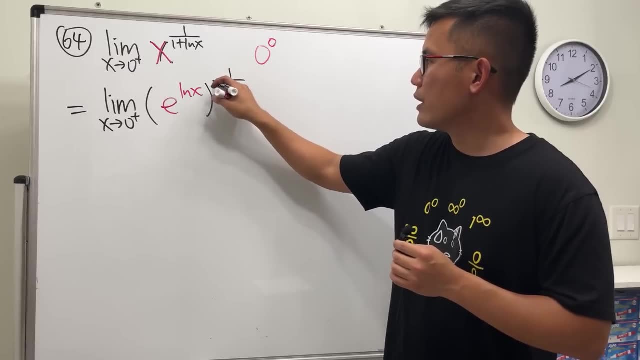 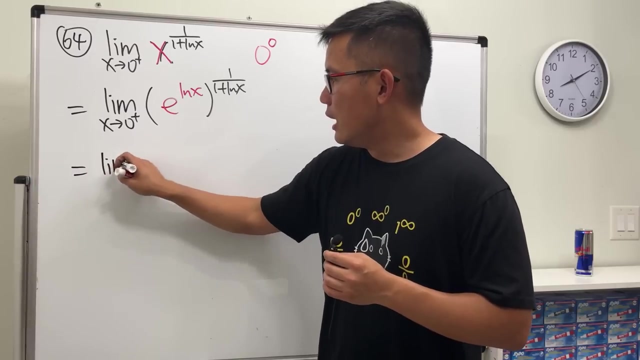 the ln x. so this right here is the limit as x approaching 0 plus e to the ln x power and then raised to the 1 over 0, 1 plus ln x power. now multiply the powers, so we are getting limit as x approaching 0 plus. 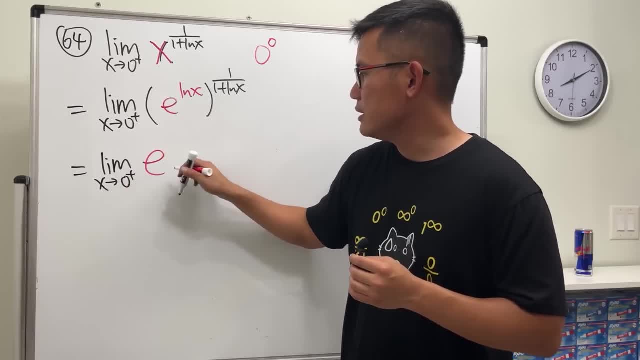 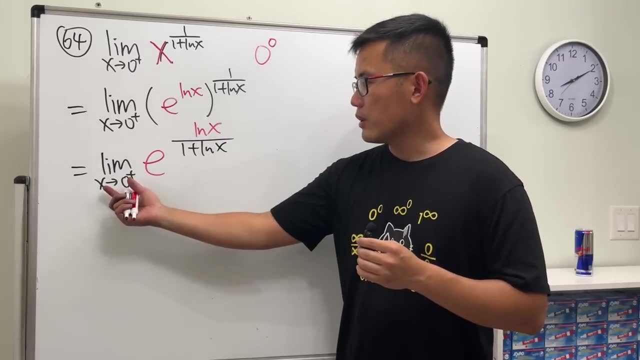 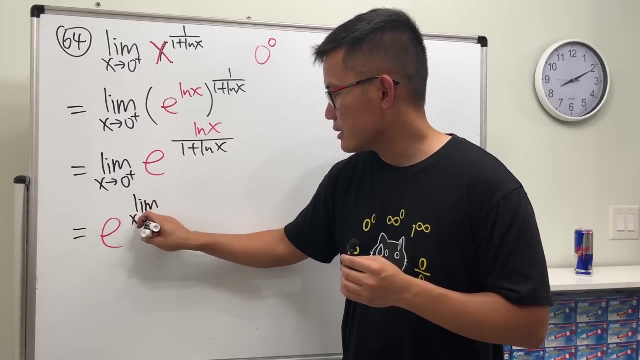 and then we have just do like this: e and then ln x over 1 plus ln x power. now just focus on doing the limits right here. so this right here is equal to e and then let's just focus on the limit as x approaching 0 plus. 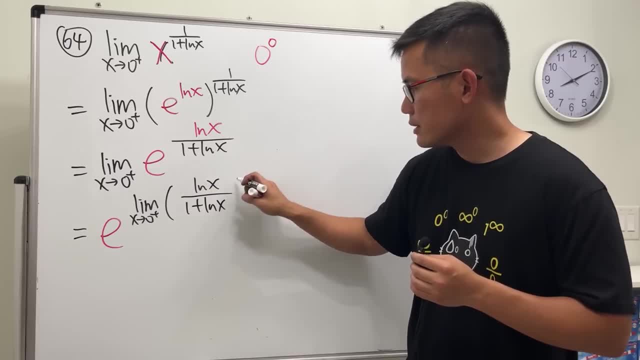 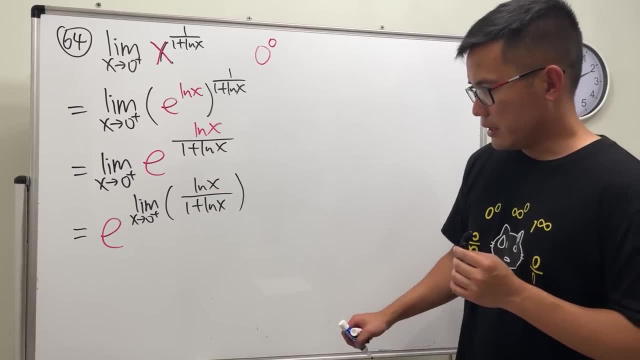 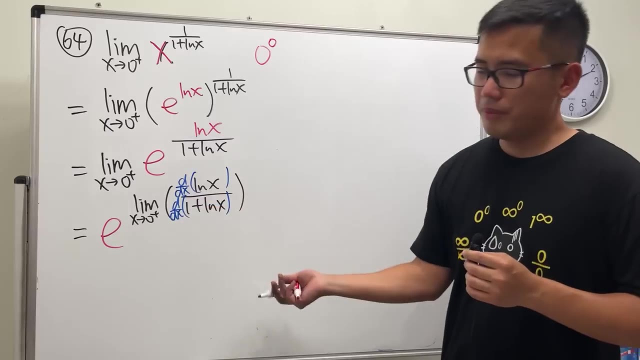 ael an x over one plus album x. but if you put 0 plus into here and here we get negative infinity over infinity. we can negative infinity over negative infinity. so we can use like we probably will. in fact, we can just get rid of the one, because the one doesn't matter. walk well, okay, but perhaps this is sounding more. 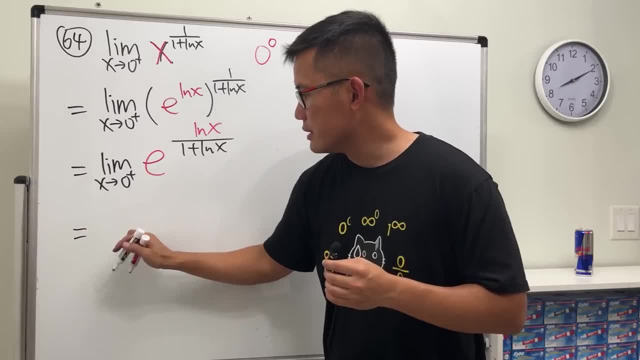 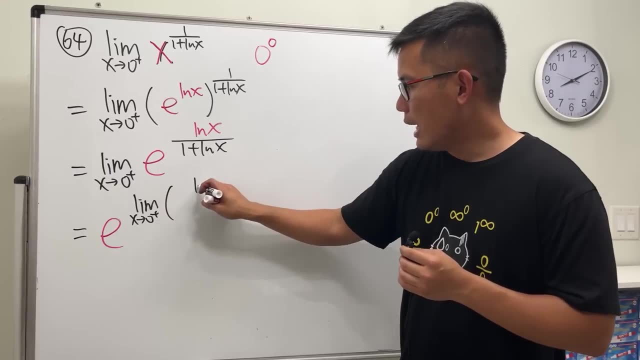 Now just focus on doing the limits right here. So this right here is equal to e. and then let's just focus on the limit as x. So this right here is equal to e, and then let's just focus on the limit as x approaching 0 plus ln x over 1 plus ln x. 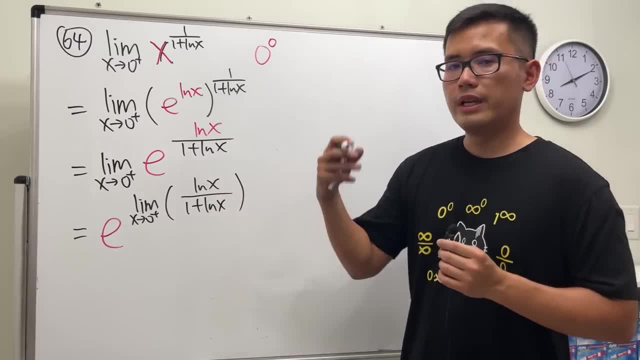 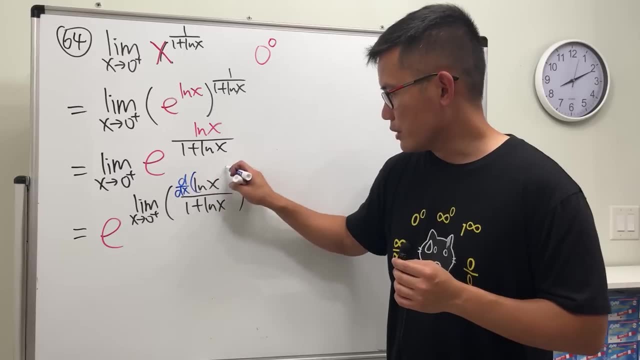 But if you put 0 plus into here and here, we get negative infinity over infinity, We get negative infinity over negative infinity. So we can use L'Hopital's rule. Well, in fact, we can just get rid of the 1, because the 1 doesn't matter when we have infinity. 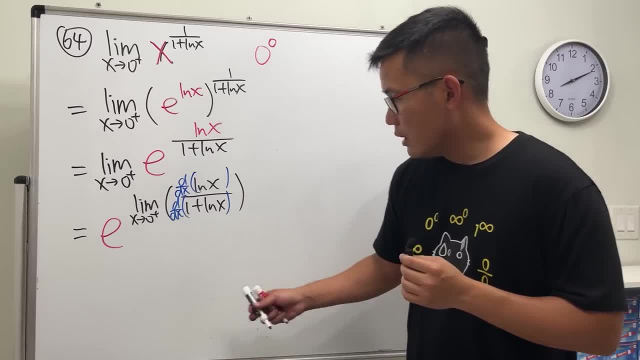 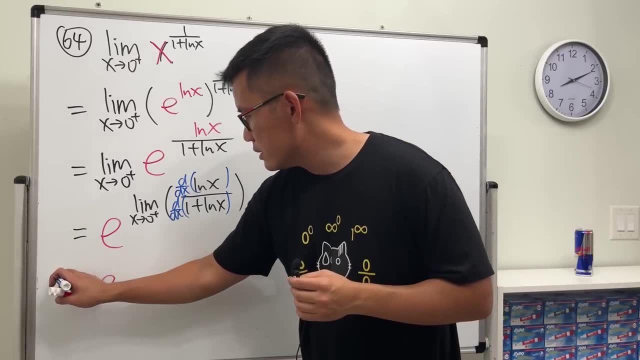 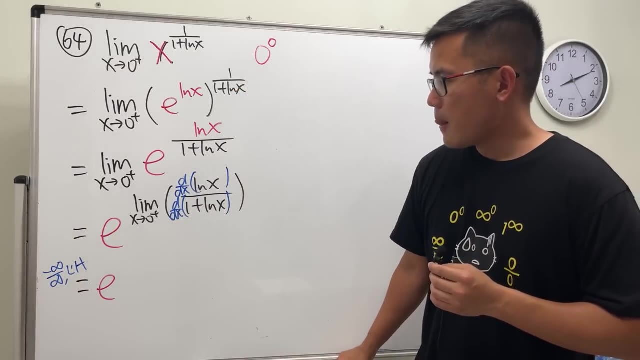 But perhaps this is slightly more legitimate. Anyway, though this right here we get e for the base, And then Again, the blue part is negative: infinity over infinity. so L'Hopital's rule, And let's do this in black. 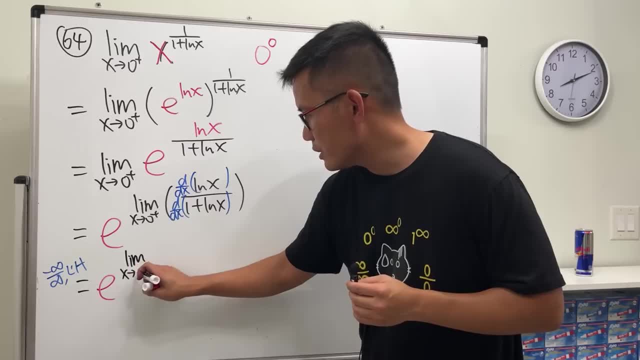 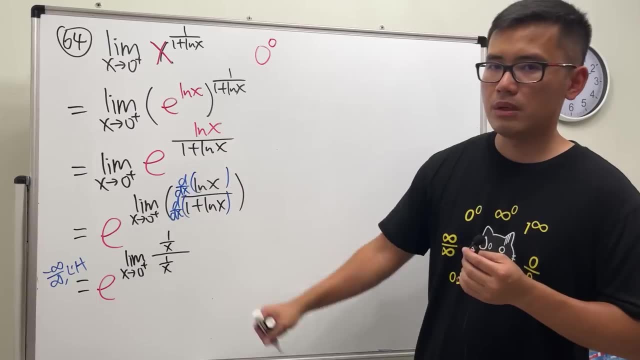 So this right here is the limit as x approaching 0 plus, The top is 1 over x. The bottom is also 1 over x, The 1 doesn't matter, They cancel, Just 1.. So on all, the answer is e. 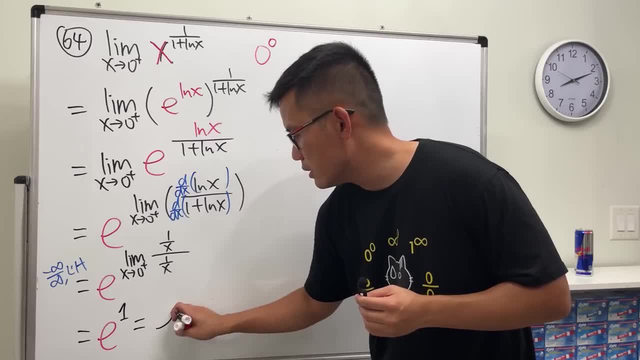 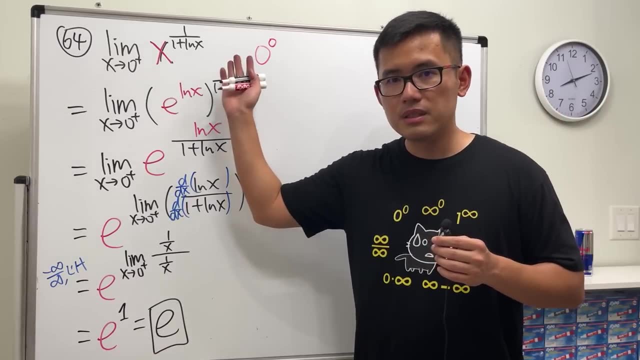 To the 1,, which is just e. 0 to the 0th power, we end up with e. This is the limit, So limit in determinant form. we can get some other numbers besides 1.. It's not like there's no agreement. 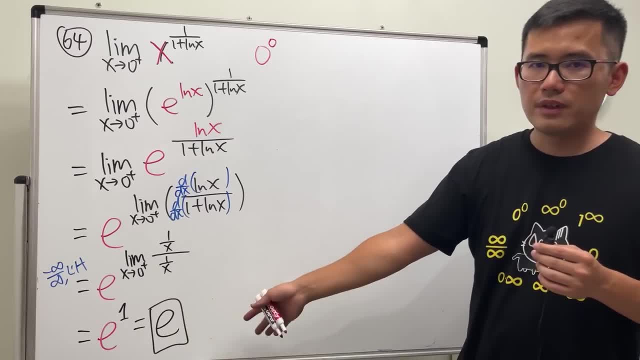 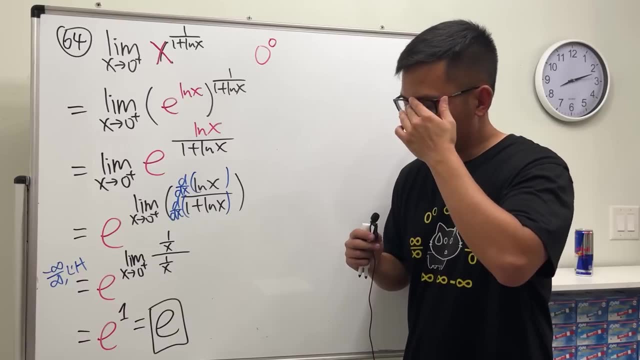 This question. everybody will agree that the answer is e 2.718-ish, So there will be no argument for this one right here. Everybody will be happy. If you go to people's birthday party, do not show them 0 to the 0th power. 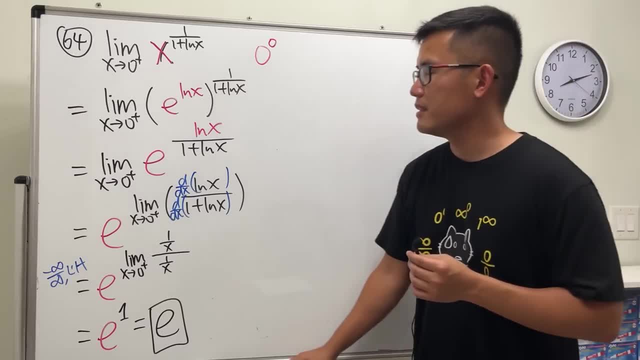 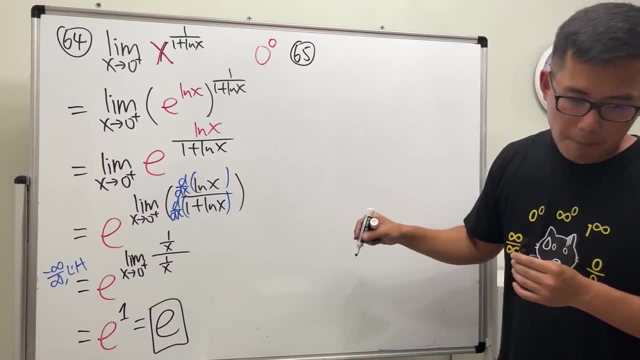 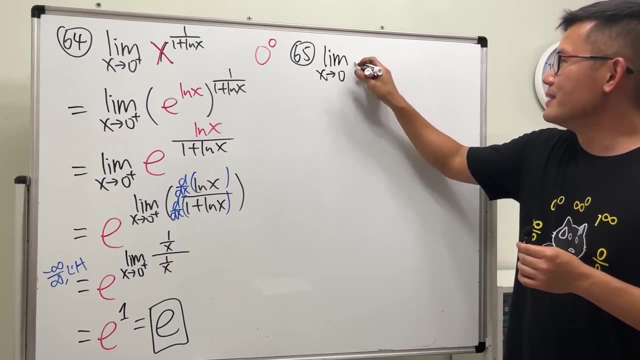 Show them this limit and you will be invited. That's the idea Number 65. The limit as x approaching 0. Finally, It's just 0. Anyway, x, e to the x, over e to the x, And then minus 1.. 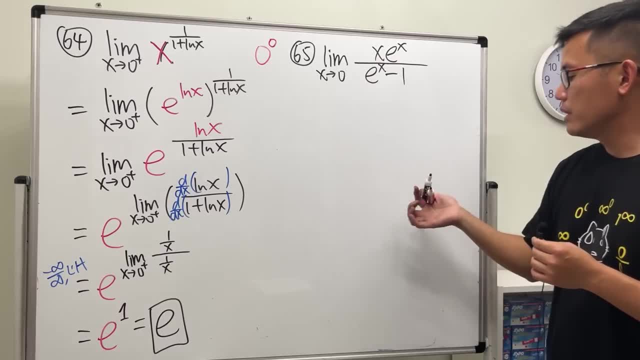 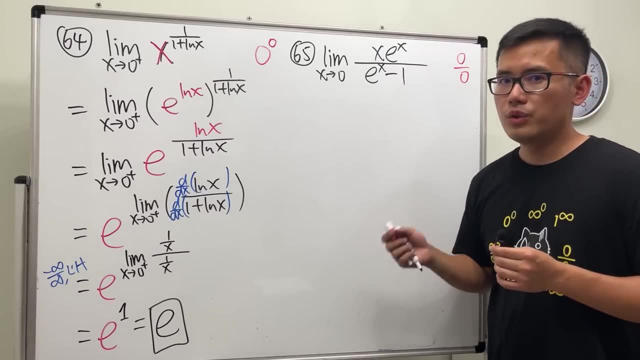 So we plug in 0. Well, no, That will give us 0 over 0.. No good, What do we do though? Hey, hey, hey, Lafiteau's rule. right now You could, but let's make it slightly easier. 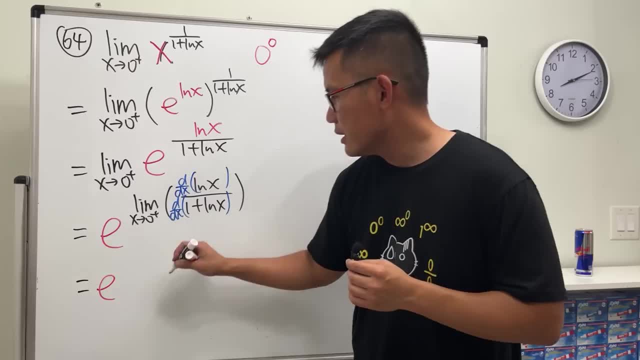 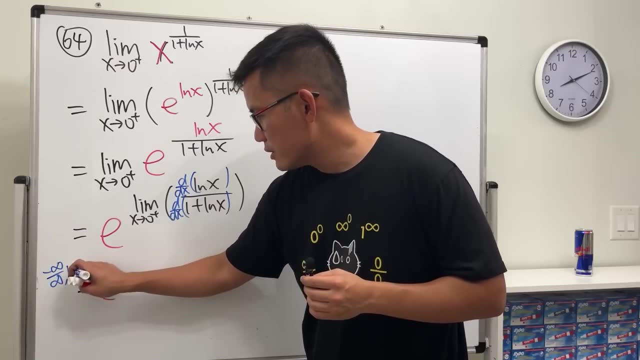 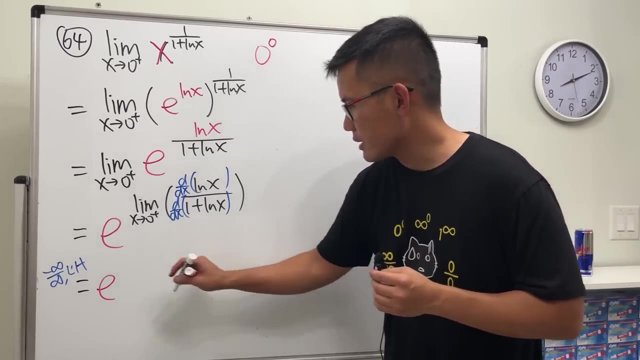 legitimate anyway, though this- right here we get e for the base, and then again the blue part is- is negative infinity over infinity. so Lapiteau's rule: Let's do this in black. So this right here is the limit as x approaching 0+. 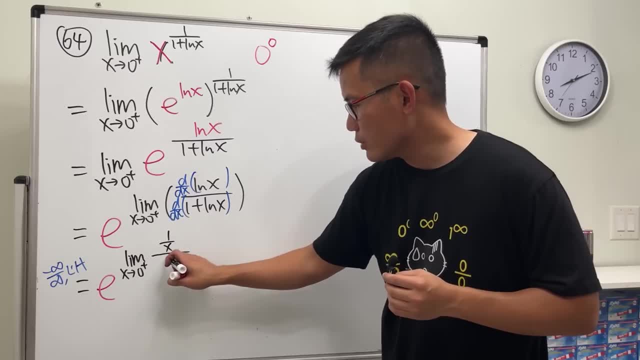 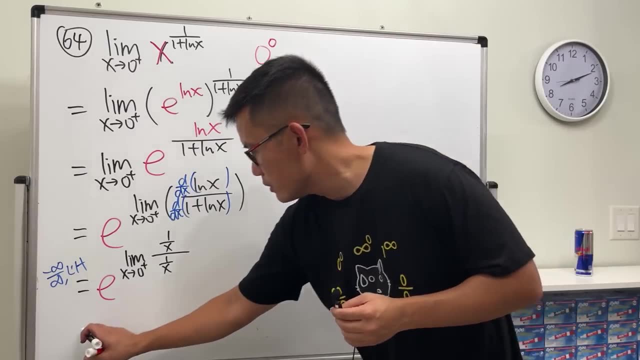 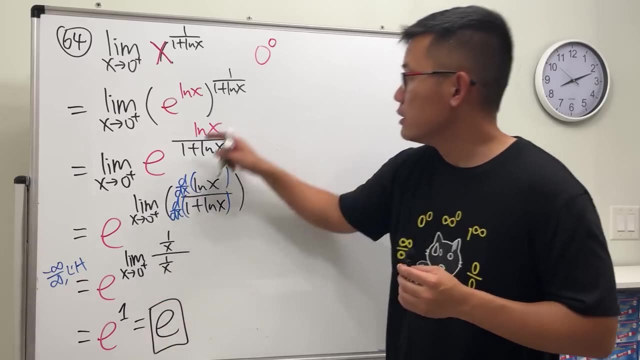 The top is 1 over x. The bottom is also 1 over x, The 1 doesn't matter, They cancel just 1.. So, all in all, the answer is e to the 1, which is just e 0 to the 0's power. we end up with e. 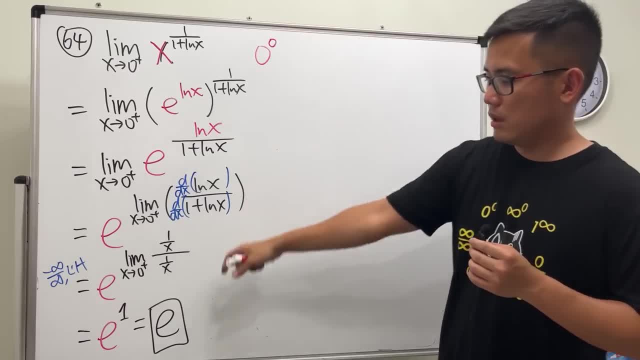 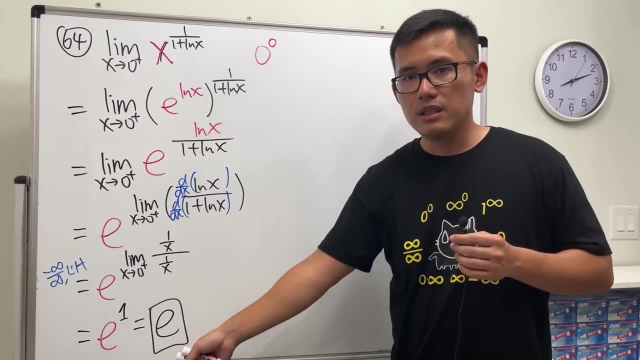 This is the limit, So limit in determinant form. we can get some other numbers besides 1.. It's not like there's no agreement This question. everybody will agree that the answer is e 2.71a-ish. So there will be no argument for this one, right here. 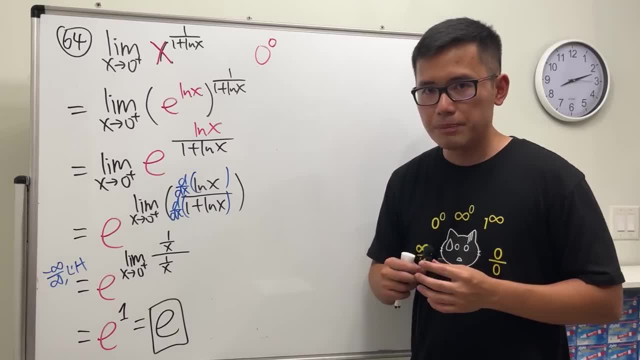 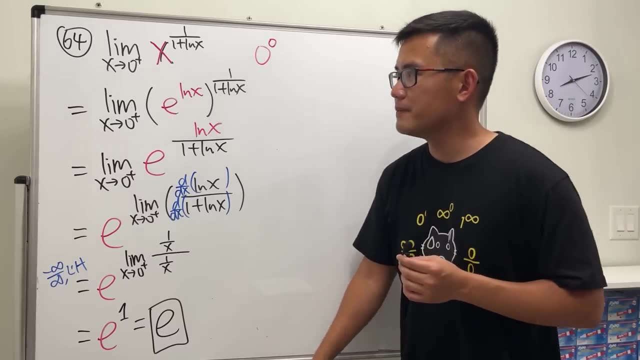 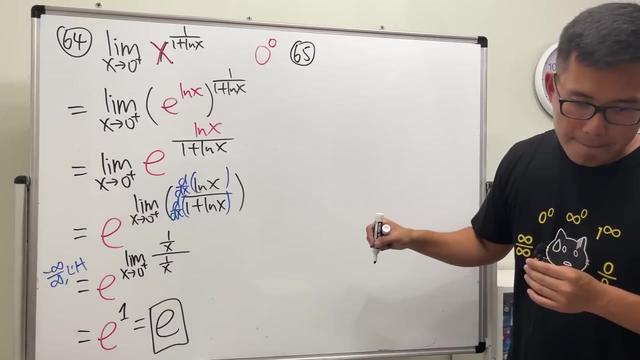 Everybody will be happy. If you go to people's birthday party, do not show them 0 to the 0's power. Show them this limit and you will be invited. That's the idea Number 65.. The limit has x approaching 0.. 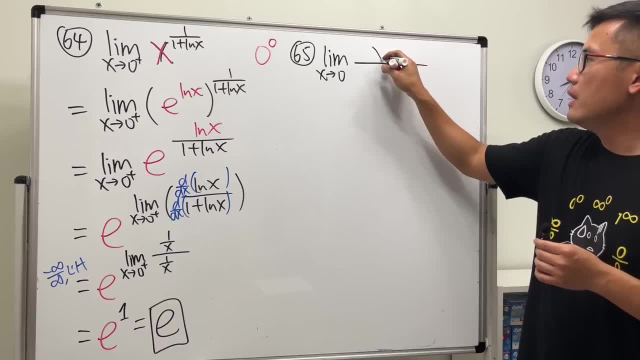 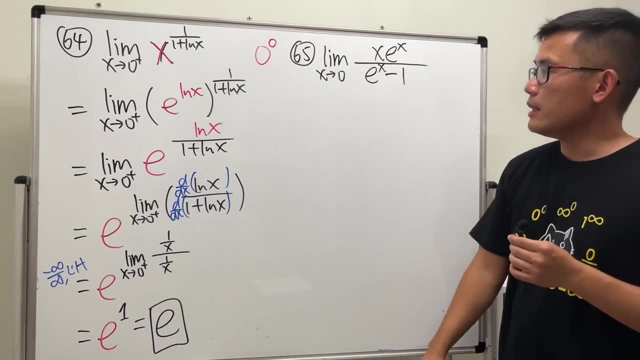 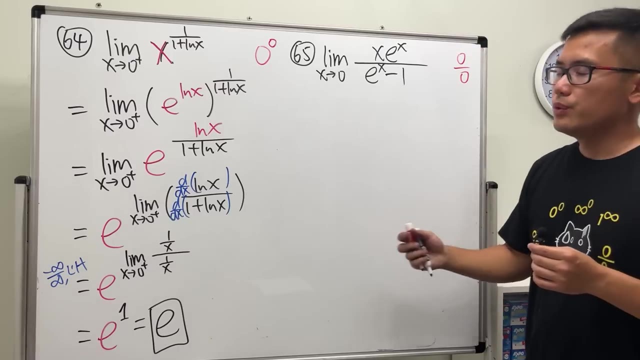 Finally It's just 0.. Anyway, x, e to the x, over e to the x, And then minus 1.. So we plug in 0, but no, That will give us 0 over 0.. No good, What do we do though? 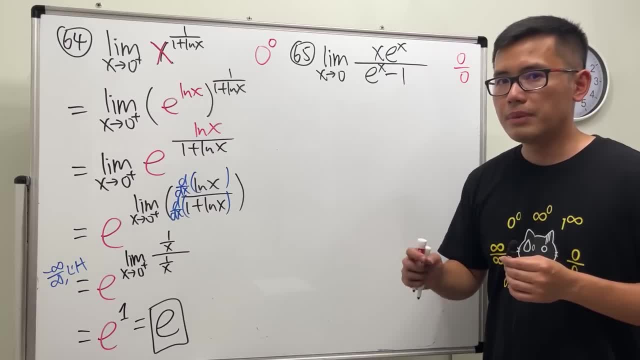 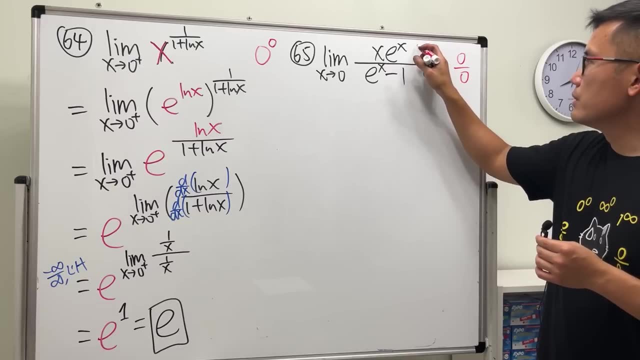 Hey, hey, hey, Lafitteau's rule. right now You could, but let's make it slightly easier. Let's divide the top and bottom by e to the x, because they all have e to the x, So I'm just going to divide this by e to the x. 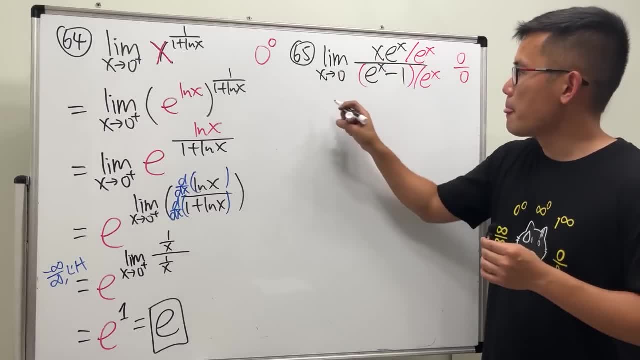 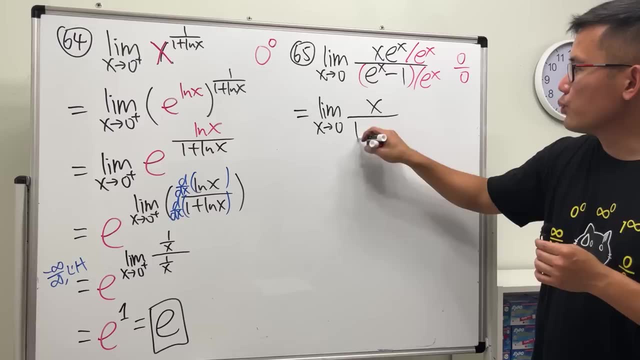 Likewise, divide this by e to the x And you'll see We get limit as x approaching 0. They cancel Reduce is 1.. 1 over e to the x- That's right here- as e to the negative x. 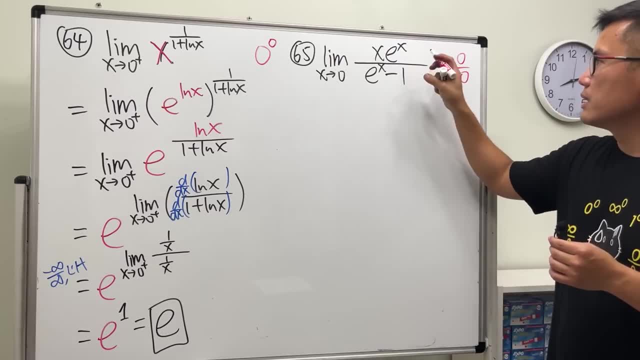 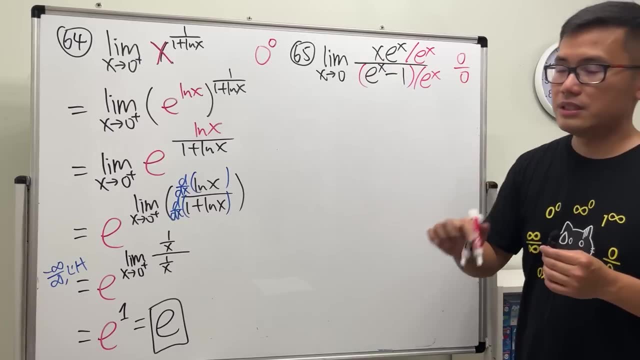 Let's divide the top and bottom by e to the x, Because they all have e to the x, huh, So I'm just going to divide this by e to the x. Likewise, divide this by e to the x And you'll see. 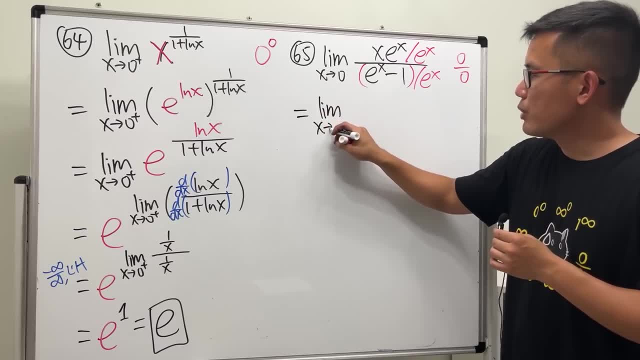 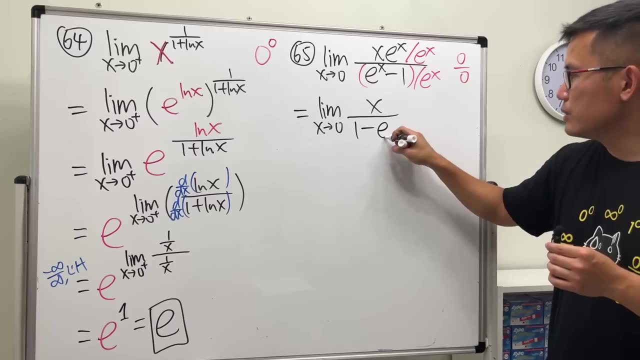 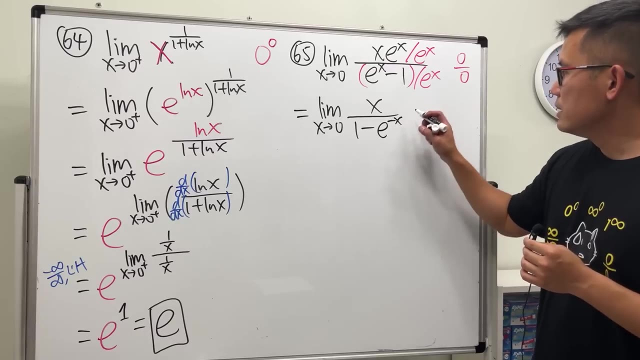 We get limit as x approaching 0. They cancel. Reduce is 1.. 1 over e to the x, That's ready as e to the negative x. Do we really need to use Lafiteau's rule? No, Because now we can see this is just 0 over. 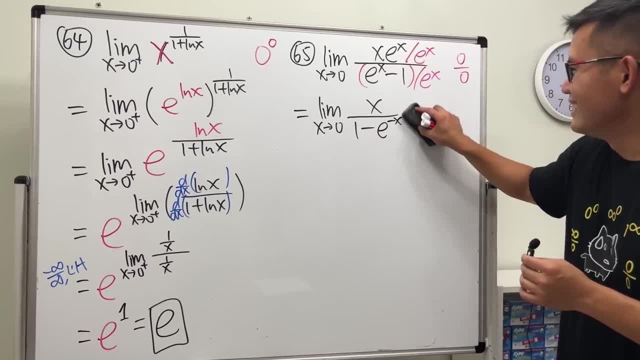 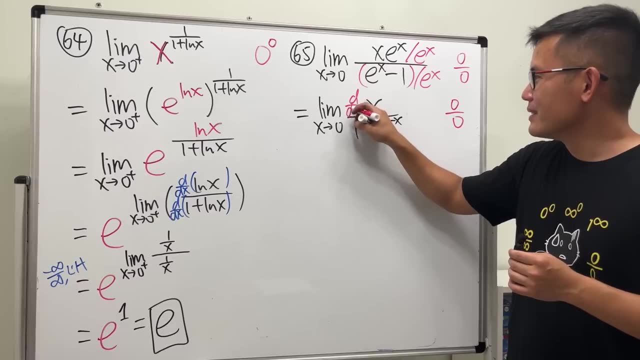 No, no, no, We still have to use Lafiteau's rule. We still end up with 0 over 0 right here. So yeah, We still need to use Lafiteau's rule. So here we go, d dx. 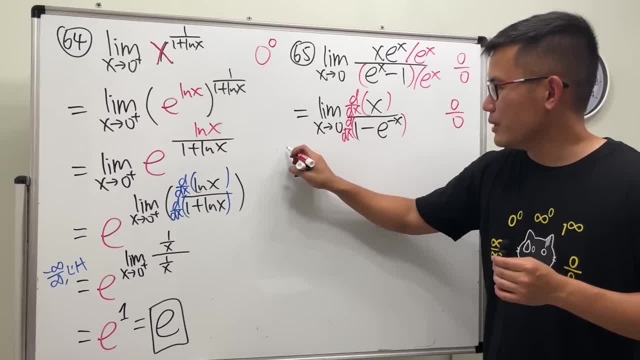 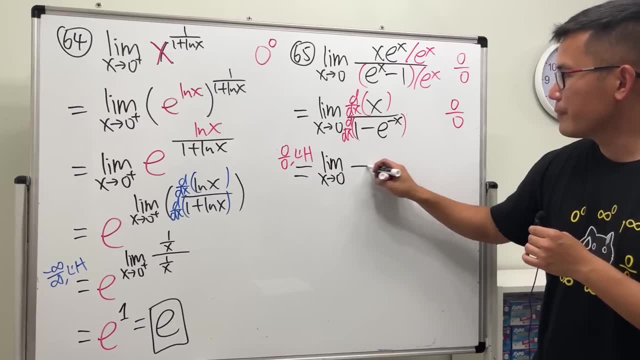 d, dx. The Lafiteau's rule is much easier than this. Let's do it this way though: 0 over 0.. Lafiteau's rule, So limit as x approaching 0.. Derivative x is 1.. 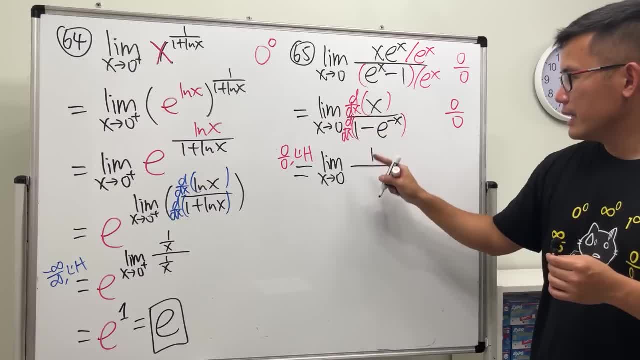 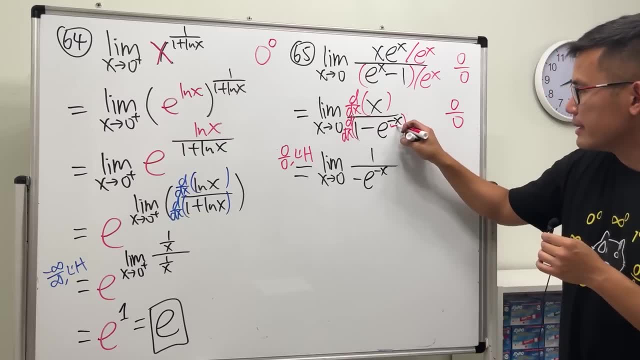 Derivative 1 is 0.. Derivative of negative e to the negative x is negative e to the negative x. But we will use the chain rule. Multiply by this derivative, which is negative 1.. So it's actually positive e to the negative x. 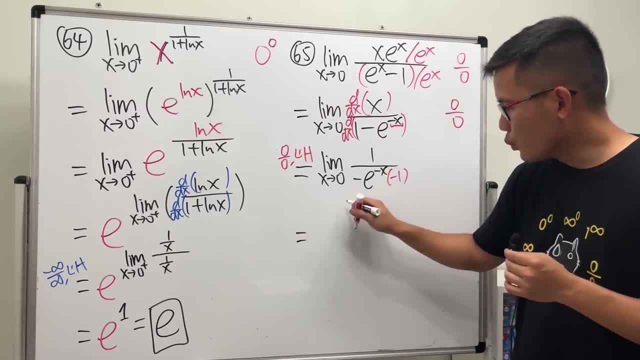 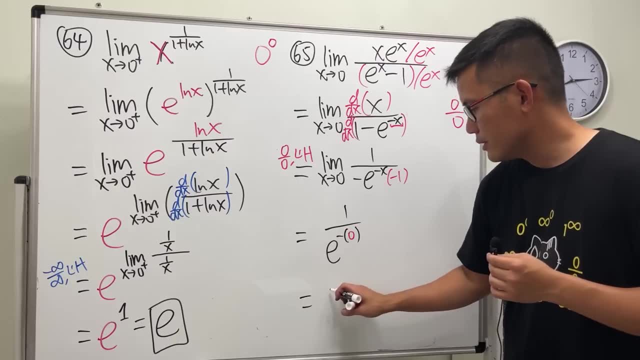 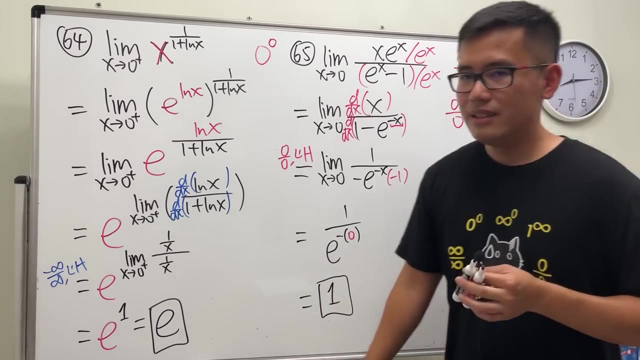 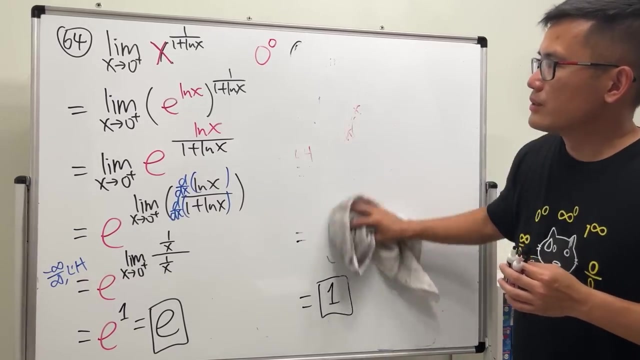 But then if you put 0 into here, You will get 1 over e to the negative 0. Just 0.. Final answer is 1.. Yeah, 0 over 0.. Yes, It can also be 1.. It can also be 1.. 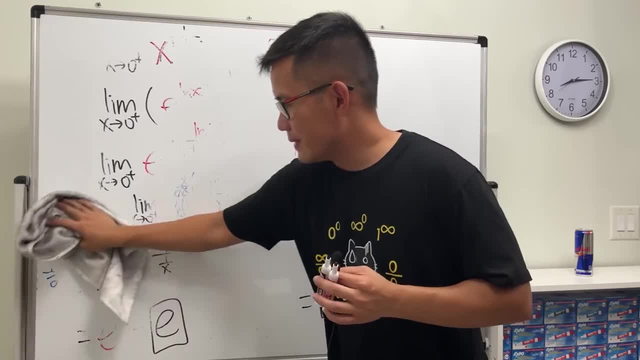 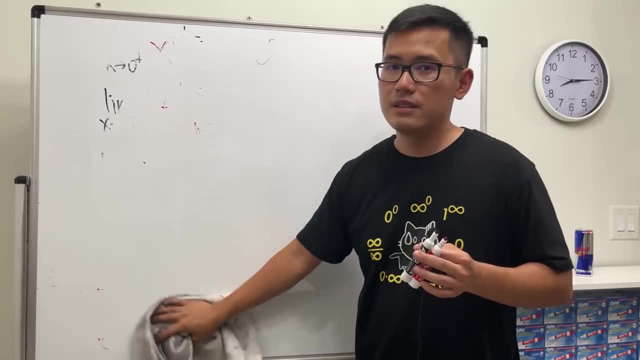 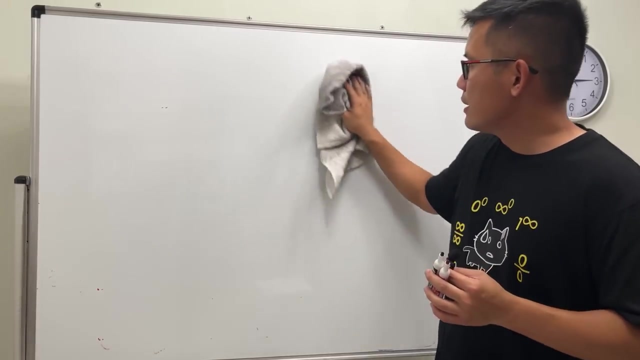 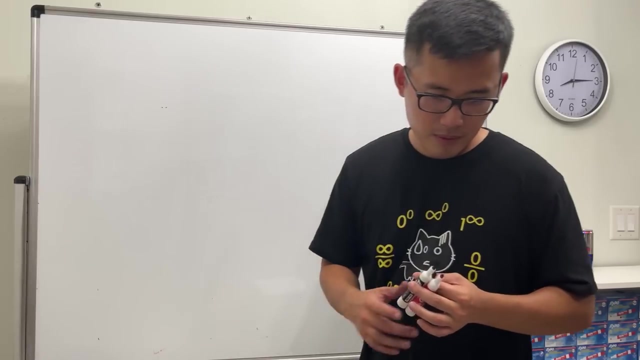 So hopefully you guys are getting all the things that you have to worry about And you can see that all the things that you have to be careful And all the techniques- And these are not the hardest part yet. Okay, Number 66.. 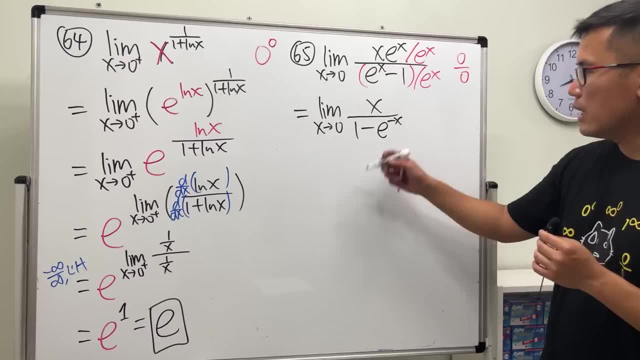 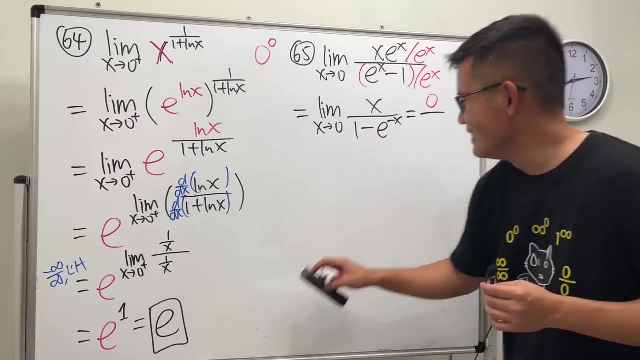 Do we really need to use Lafitteau's rule? No, Because now we can see: this is just 0 over No. no, no, We still have to use Lafitteau's rule. We still end up with 0 over 0, right here. 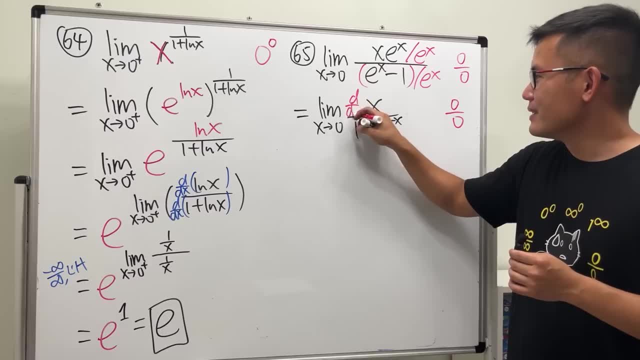 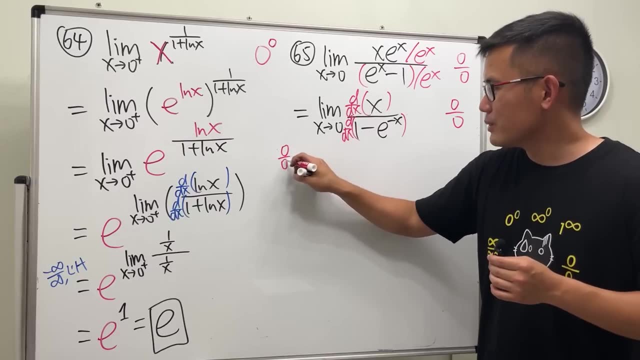 So, yeah, We still need to use Lafitteau's rule. So here we go: d dx, d dx. The Lafitteau's rule is much easier this way, though: 0 over 0.. Lafitteau's rule. 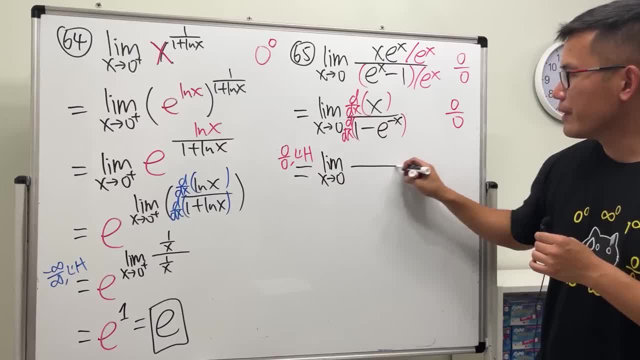 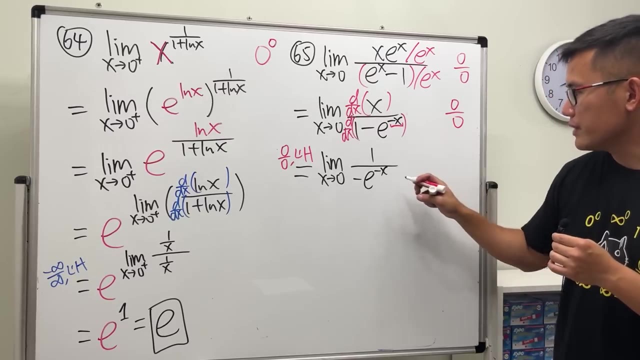 So limit as x approaching 0. Derivative x is 1.. Derivative 1 is 0.. Derivative of negative e to the negative x is negative e to the negative x, But we are using the chain rule multiplied by this derivative, which is negative 1.. 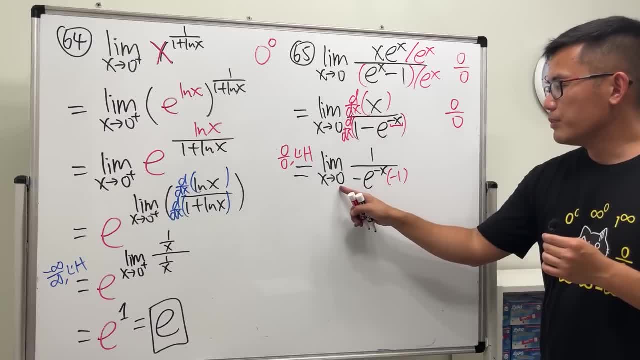 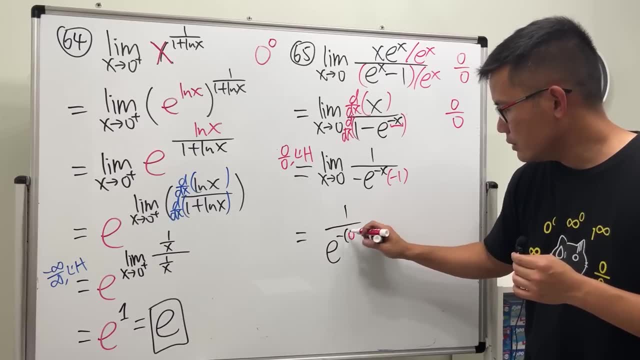 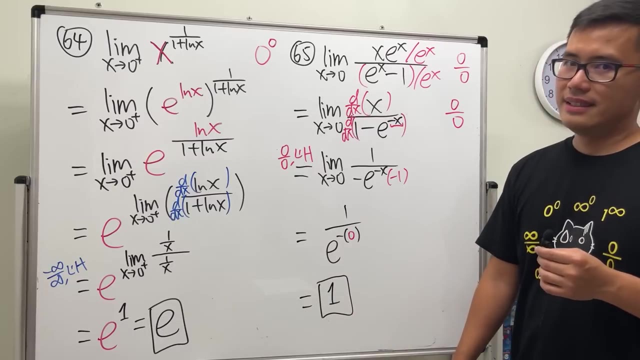 So it's actually positive e to the negative x. But then if you put 0 into here, we will get 1 over e to the negative 0. Just 0.. It's the final answer. It's 1.. Yeah, 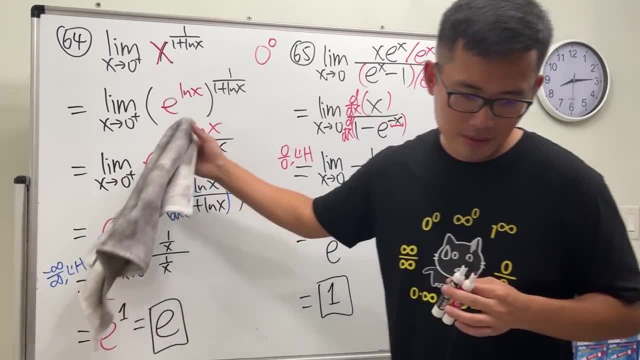 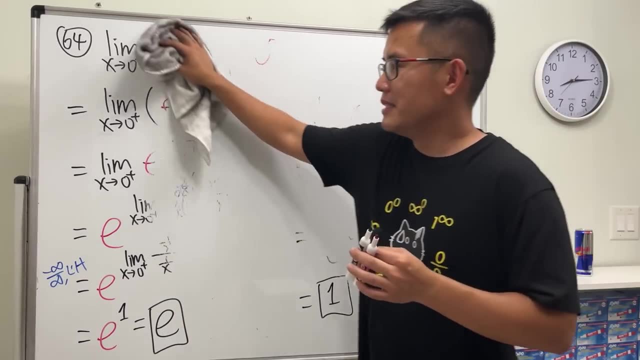 0 over 0.. Yes, It can also be 1.. It can also be 1.. So hopefully you guys are getting like all the things that you have to worry about. So hopefully you guys are getting like all the things that you have to worry about. 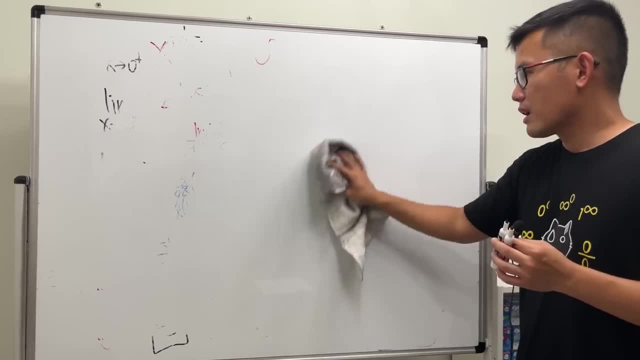 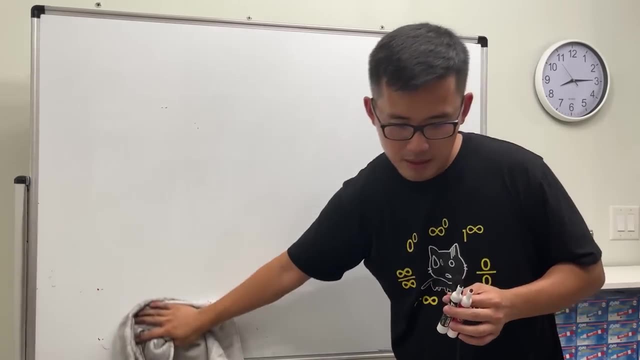 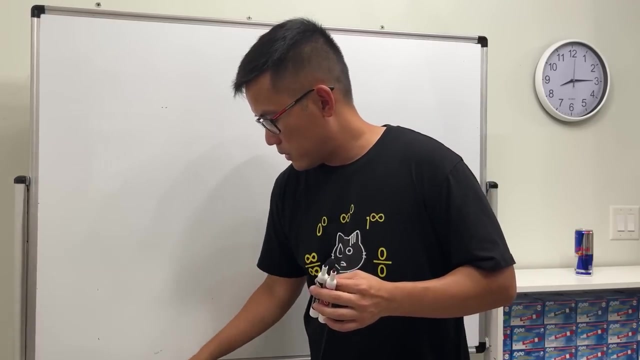 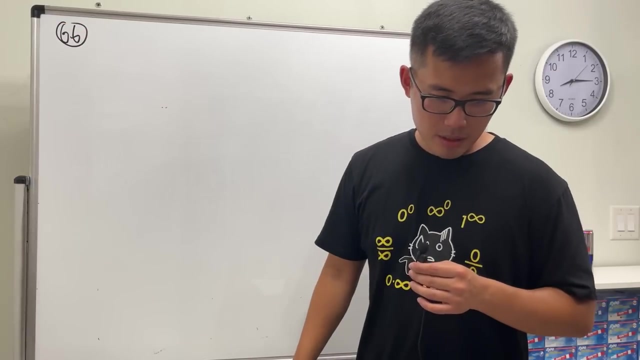 Like all the things that you have to worry about, And then you can see that all the things that you have to be careful And all the techniques- And these are not the hardest part yet. Okay, Number 66.. Limit as x approaching 0.. 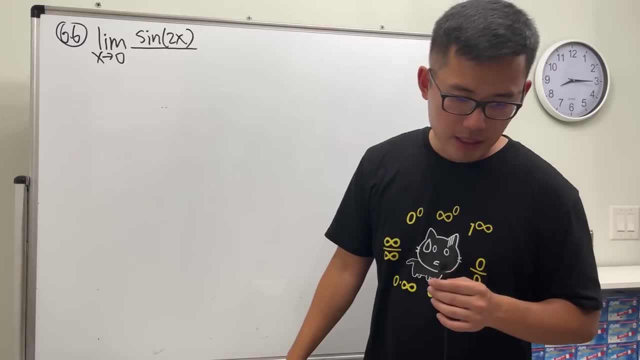 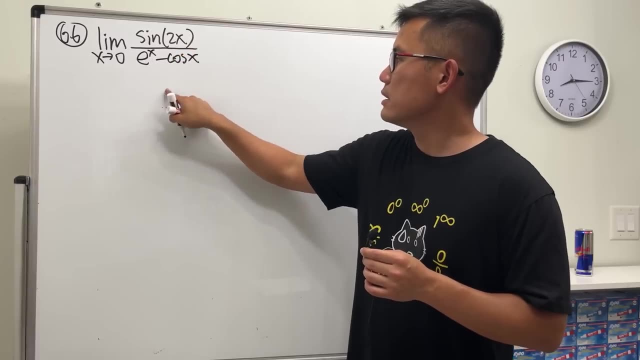 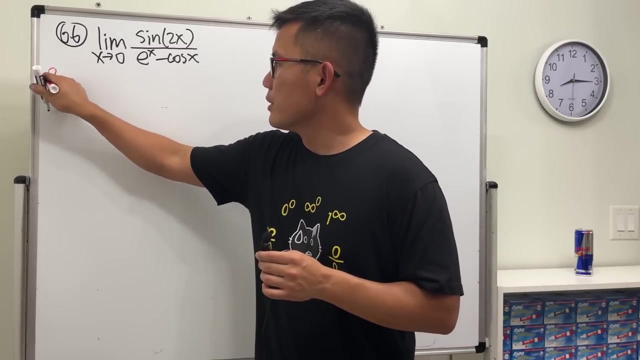 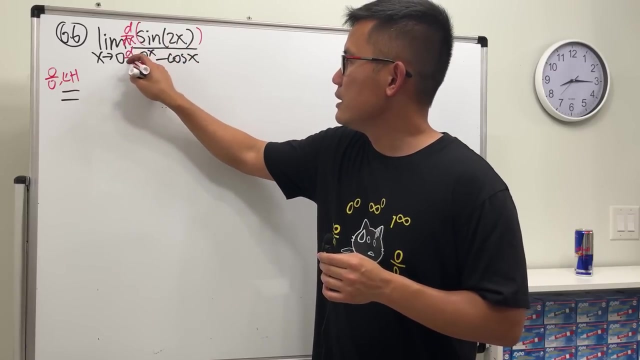 Sine of 2x and then e to the x minus cosine of x. All right, So just a quick check: 0 over 0.. So go ahead to Lafitteau's rule. So d, dx, d, dx, All right. 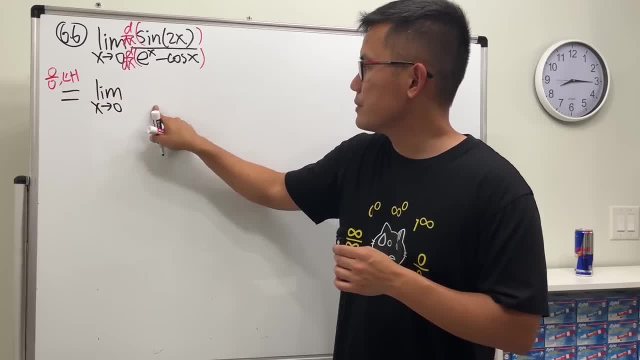 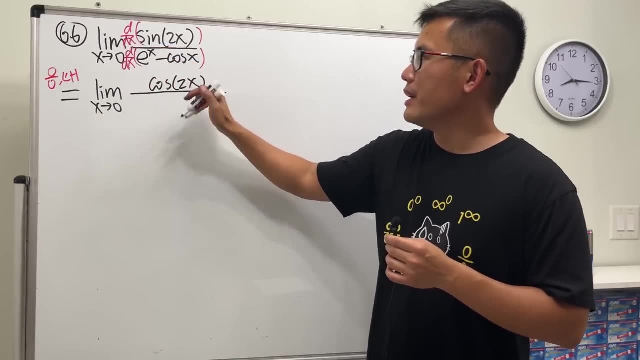 Here we have the limit as x approaching 0.. The derivative of sine is cosine- We did that today, Cool. And then multiply by the derivative of 2x, which is just a 2. So let's put that at the front. 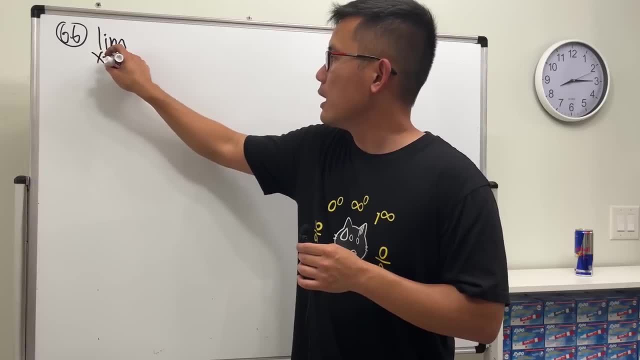 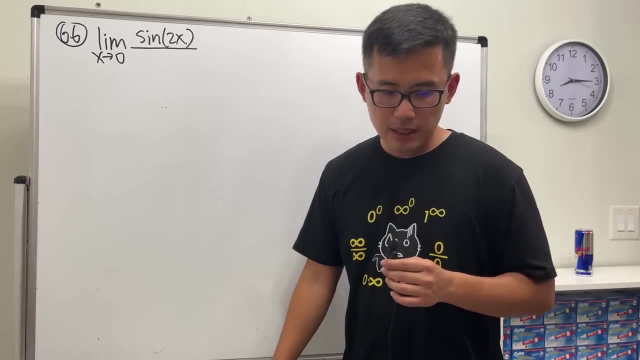 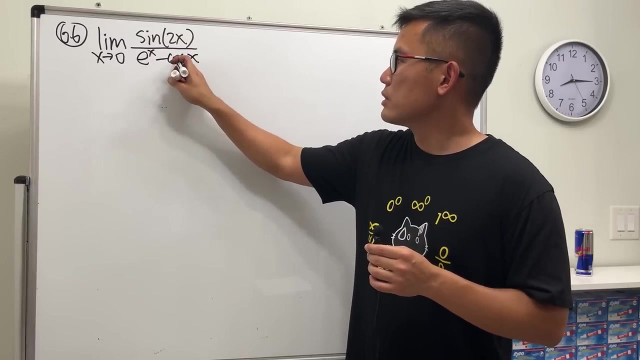 Limit as x approaching 0. Sine of 2x And then e to the x minus cosine of x. All right, So just do a quick check: 0 over 0.. So go ahead, Do L'Hospital's rule. 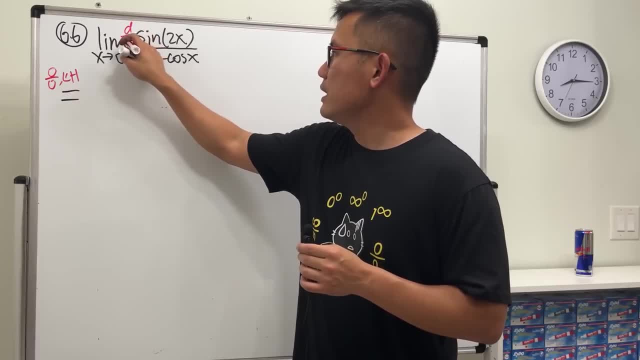 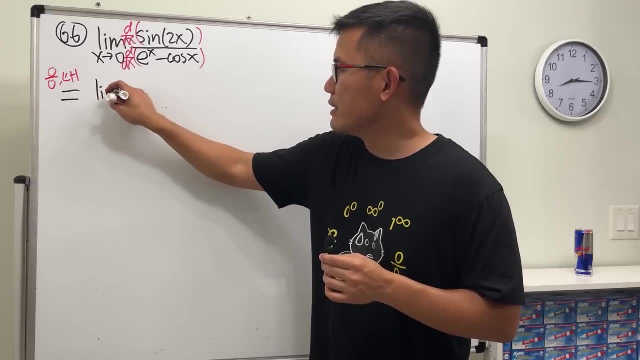 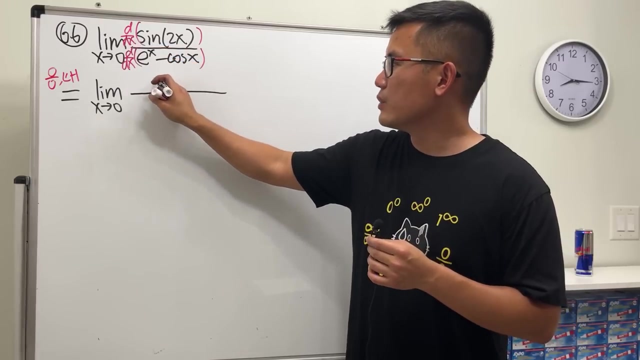 So d, dx, d, dx. All right, Here we have the limit, Here we have the limit as x approaching 0.. Derivative of sine is cosine- We did that today, Cool. And then multiply by the derivative of 2x, which is just a 2.. 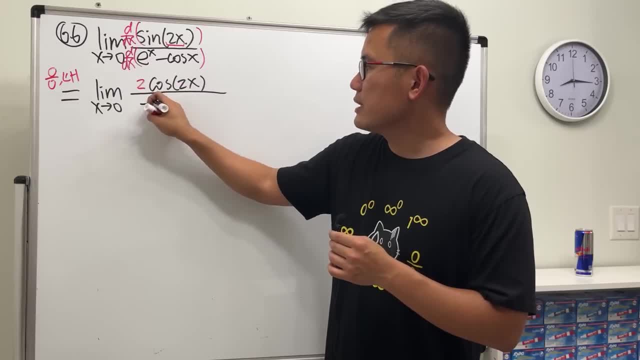 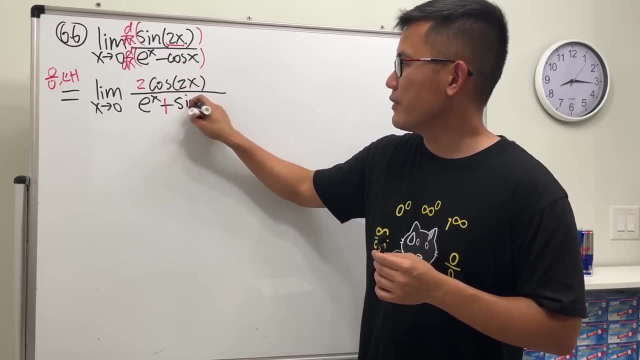 So let's put that at the front. Derivative of e to the x is e to the x. Derivative of negative cosine is negative sine. So negative times negative becomes positive, And then we have the sine x. Cool, Now put 0 into all the x's. 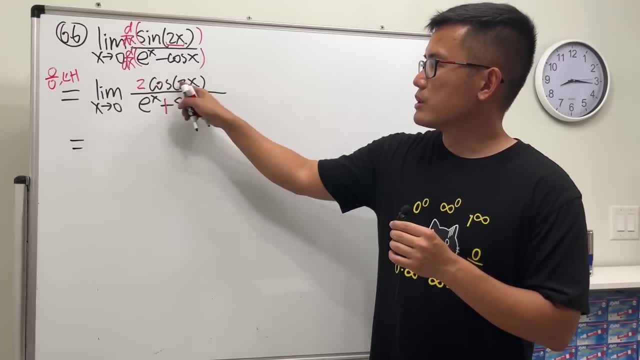 Then we get try it. Cosine of 0 is 1.. So on the top we have 2.. Put the 0 in here. E to the 0 is 1.. Sine of 0 is 1.. 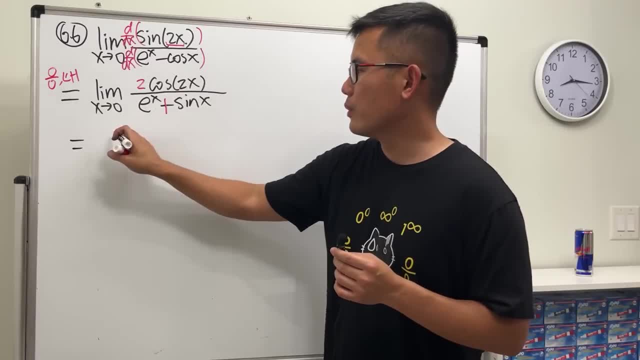 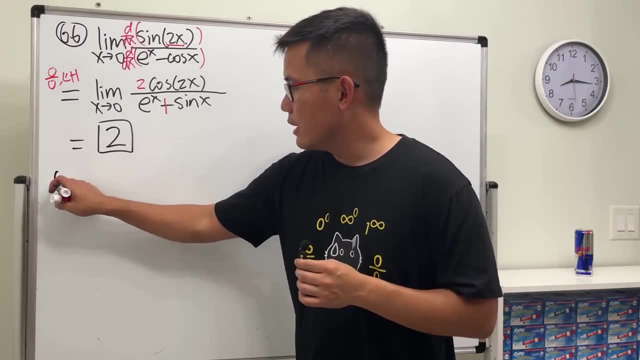 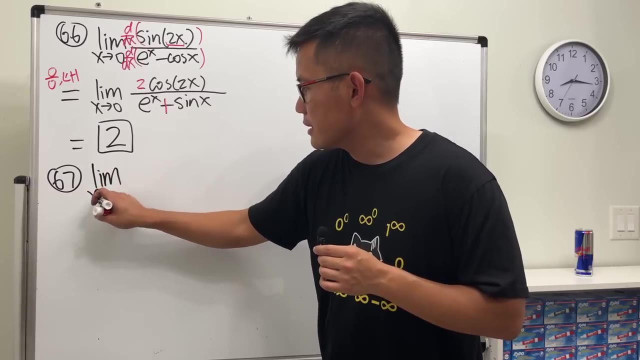 Sine of 0 is 0. So just 2 over 1, which is 2.. Done, So you can verify that on your own. 67, we have the limit as x approaching pi over 2.. And then we have secant. 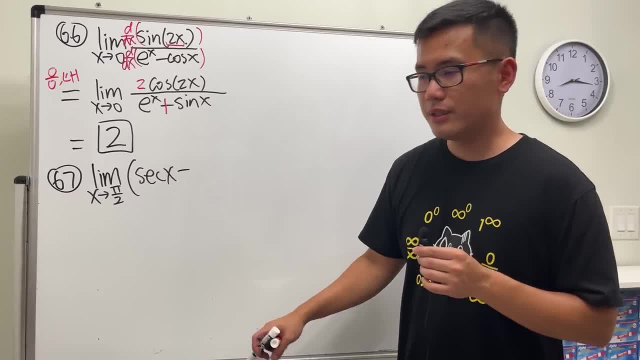 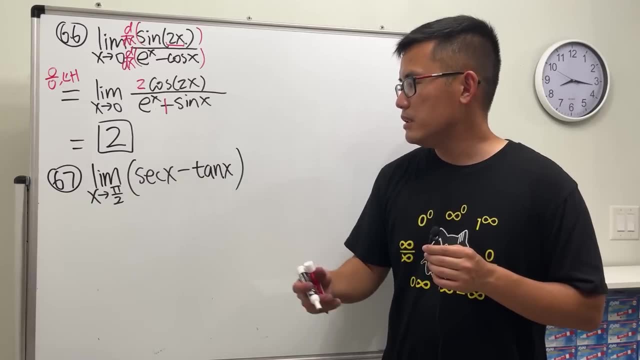 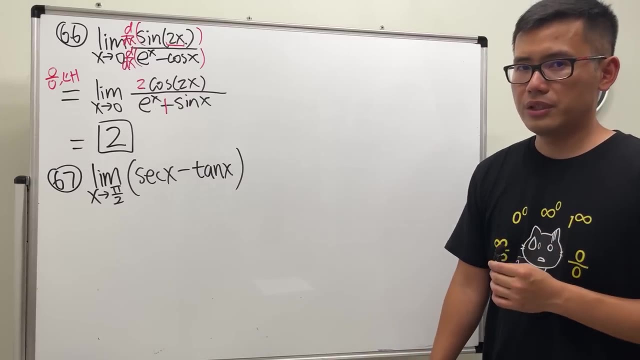 And then we have secant x minus tangent x. Wow, I'll tell you, It's an infinity minus infinity case, depending if you are talking about a plus or minus. But no, Let's combine the fraction. Wait, Where are the fractions? 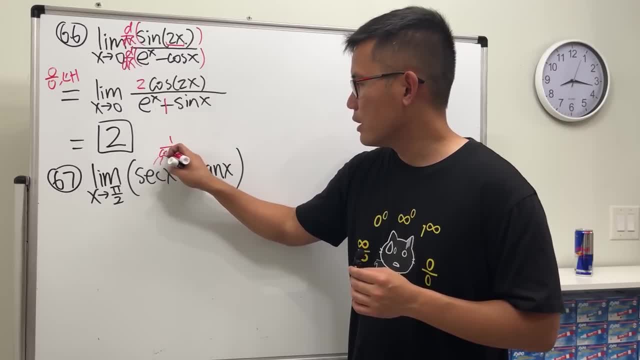 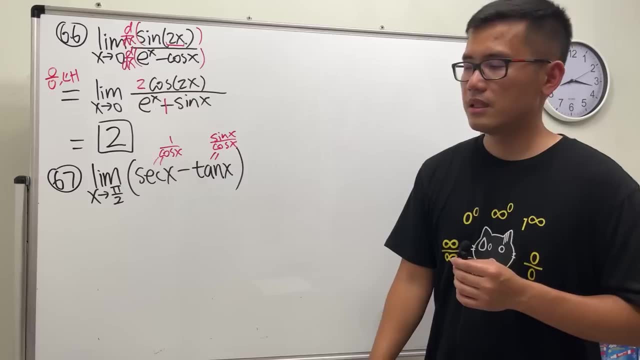 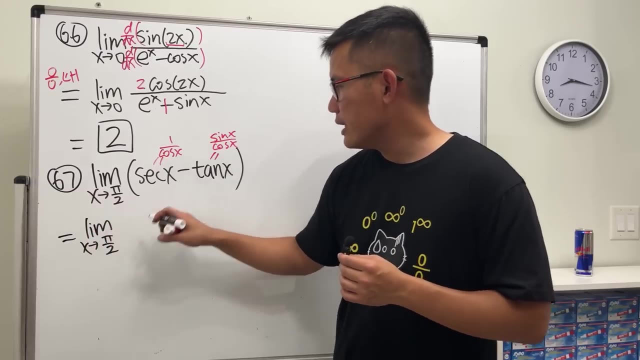 This right here, it's the same as 1 over cosine x. This right here, it's the same as sine x over 2. Cosine x, isn't it? So, all in all, this is just the limit as x approaching pi over 2.. 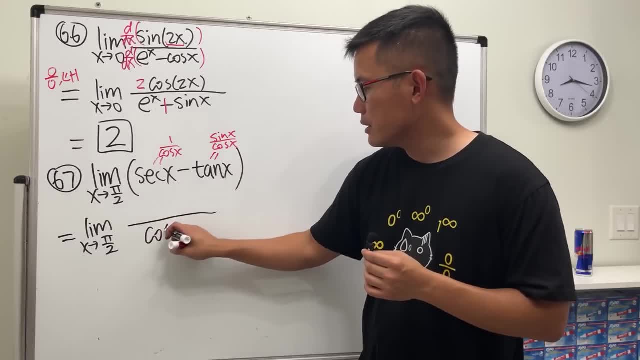 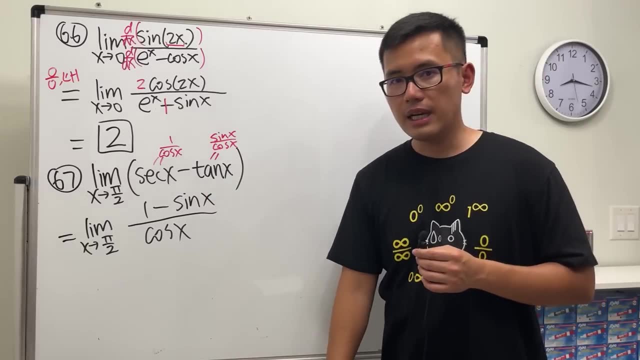 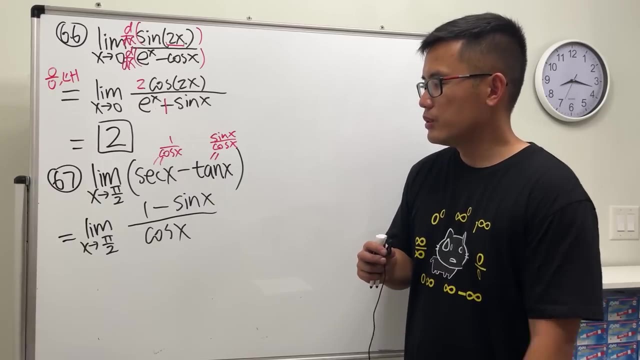 And then we have cosine x on the bottom and then 1 minus sine x on the top. Yeah, And in fact yes, we get 0 over 0. But do we really need to use L'Hopital's rule for this? 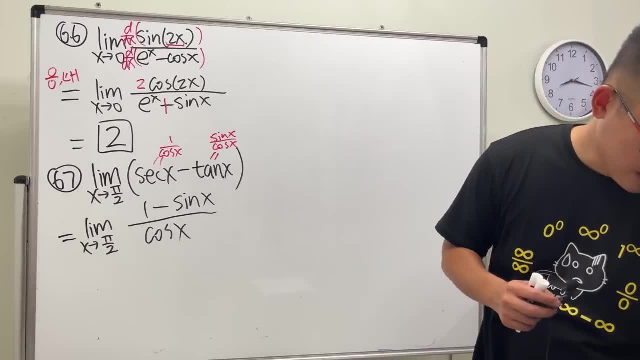 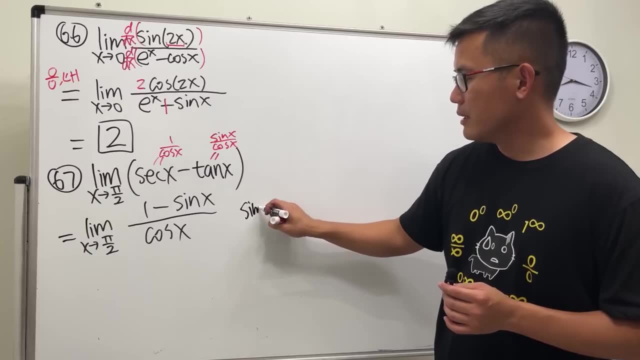 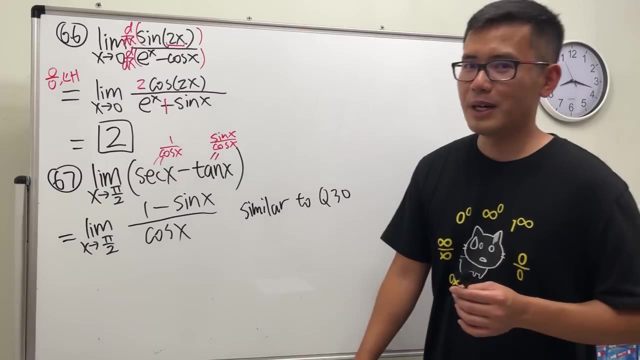 We don't, Because earlier today we did something similar to this, Question number 30, right, Similar to question 30. You guys can look back. That's like I don't know how many hours ago. But we can multiply the top and bottom by 1 plus sine x. 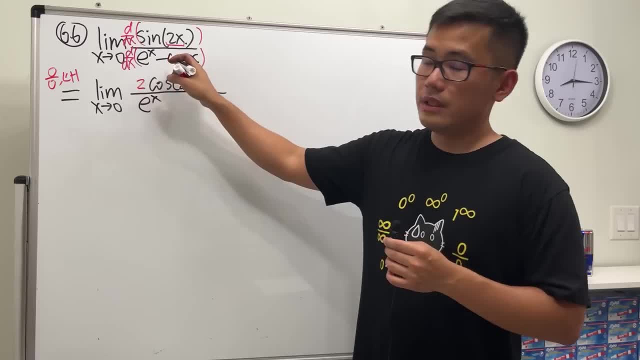 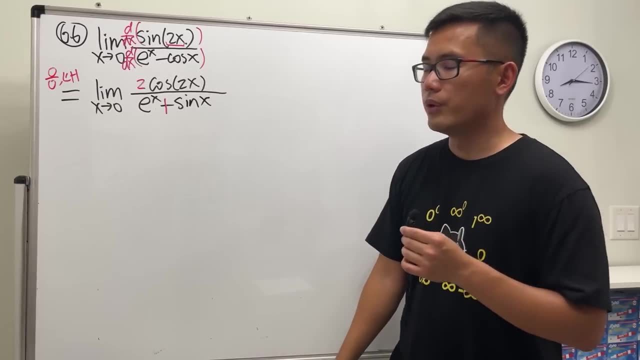 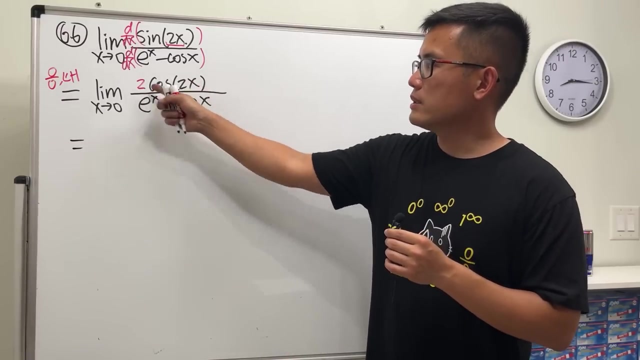 The derivative of e to the x is e to the x. The derivative of negative cosine is negative sine. So negative times negative becomes positive, And then we have the sine x. Cool, Now put 0 into all the x's, Then we get. try it. Cosine of 0 is 1. So on the top we have 2. Put. 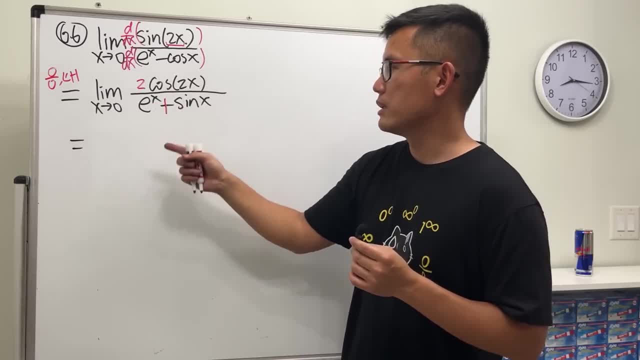 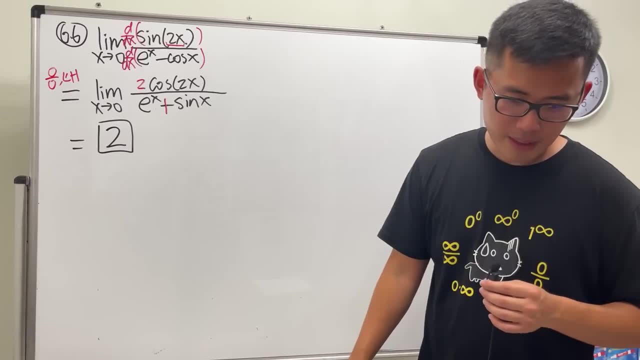 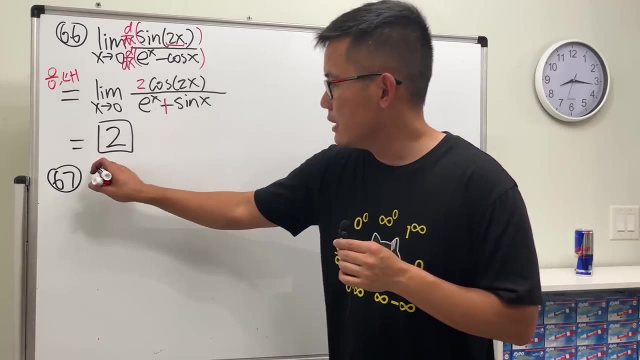 the 0 in here e to the 0 is 1.. Sine of 0 is 1.. Sine of 0 is 0. So just 2 over 1, which is 2.. Done, So you can verify that on your own. 67, we have the limit As x approaching. 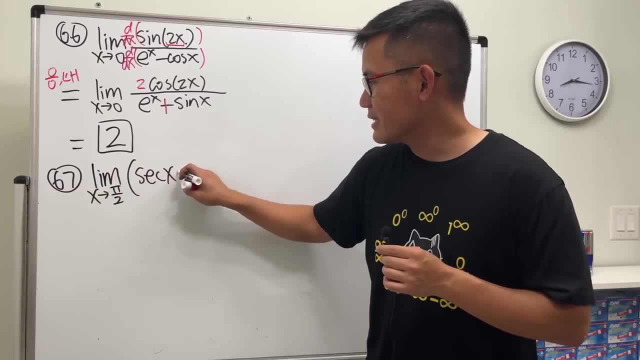 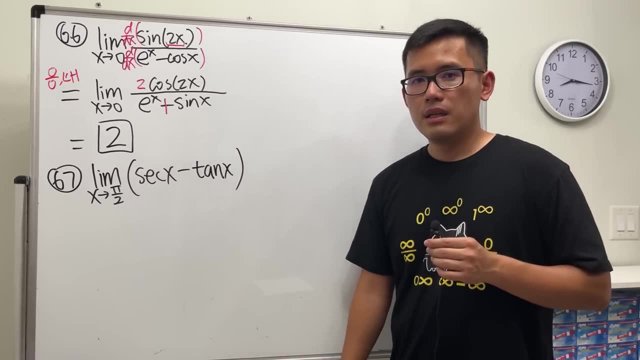 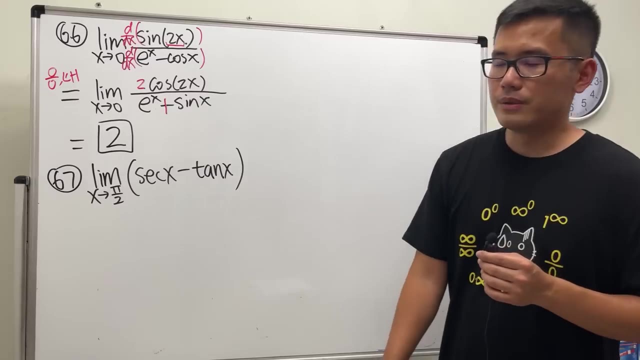 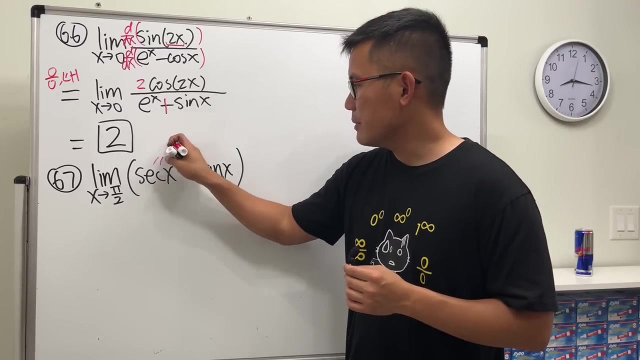 pi over 2.. And then we have secant x minus tangent x. Wow, I'll tell you, it's an infinity minus infinity case, depending if you are talking about a plus or minus. But no, let's combine the fraction. Wait, where are the fractions? This right here, it's the same as 1 over cosine. 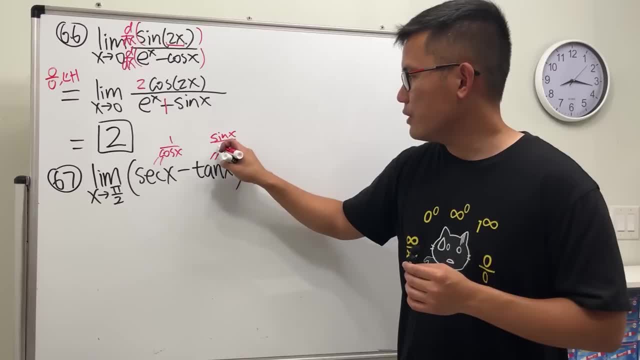 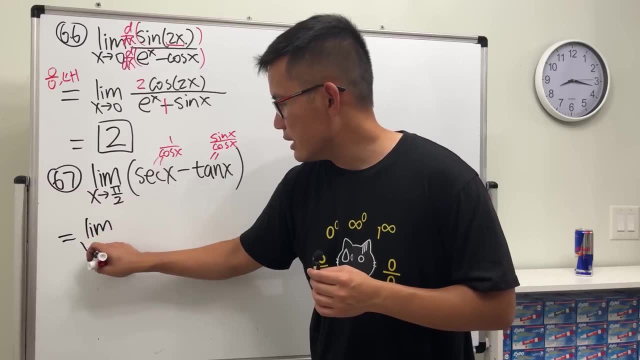 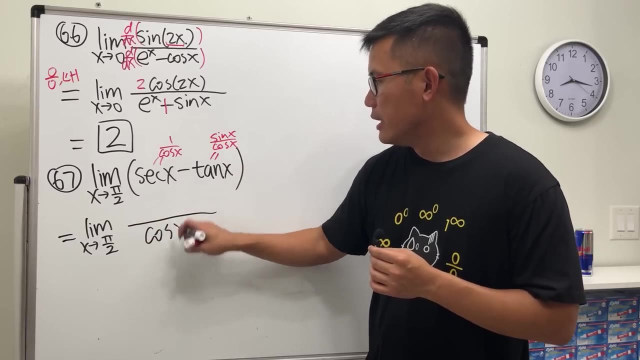 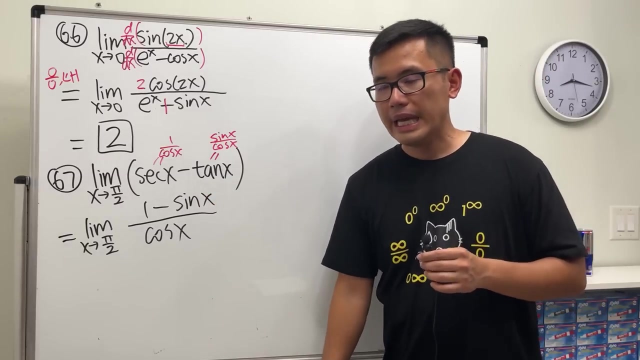 x. This right here. it's the same as sine x over 2.. Cosine x, isn't it? So all in all, this is just the limit as x approaching pi over 2.. And then we have cosine x on the bottom and then 1 minus sine x on the top. Yeah, 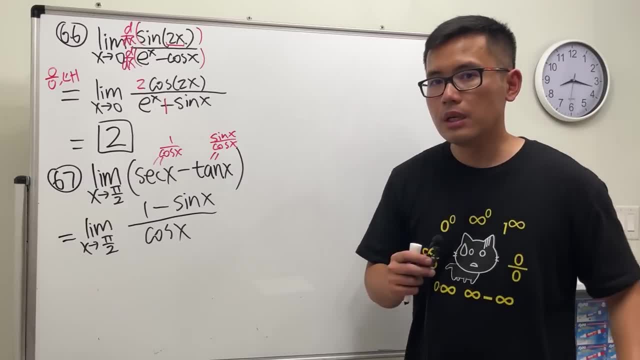 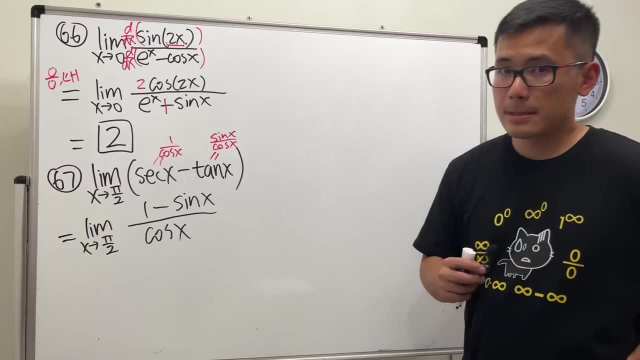 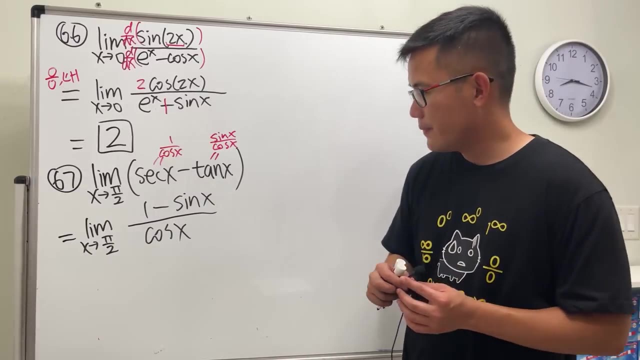 And in fact, yes, we get 0 over 0.. But do we really need to use L'Hopital's rule for this? We don't, Because earlier today we did something similar to this. Question number 30.. Similar. 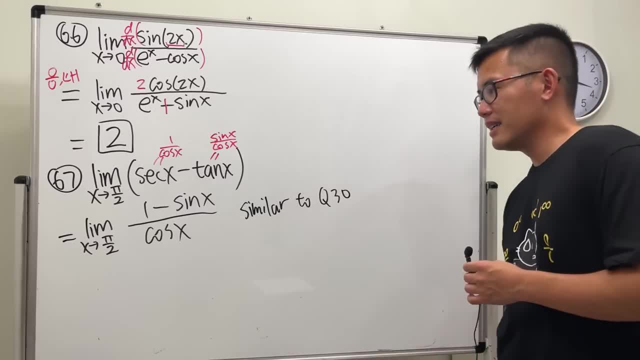 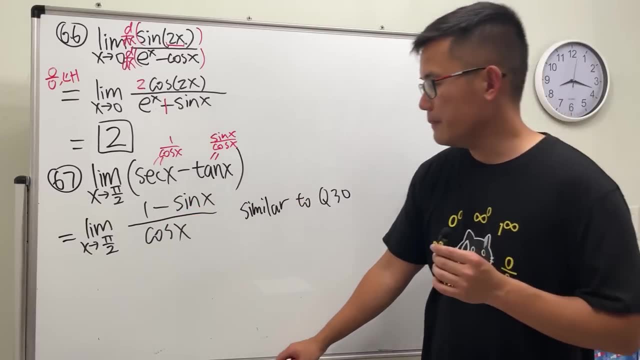 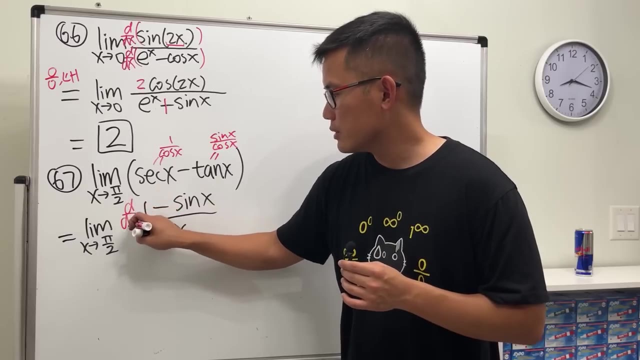 to question 30.. You guys can look back- That's like I don't know how many hours ago- But we can multiply the top and bottom by 1 plus sine x. You can do it that way, But since this is the L'Hopital's rule category, so let's just use L'Hopital's rule, Just want. 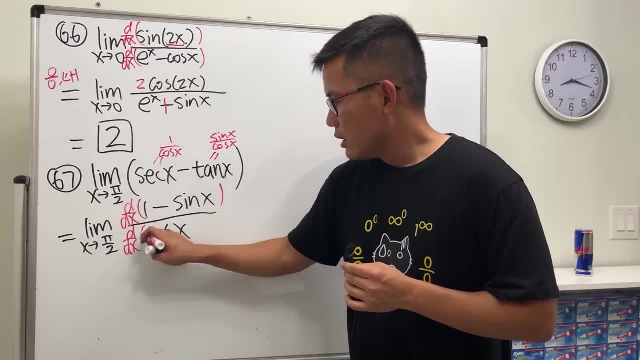 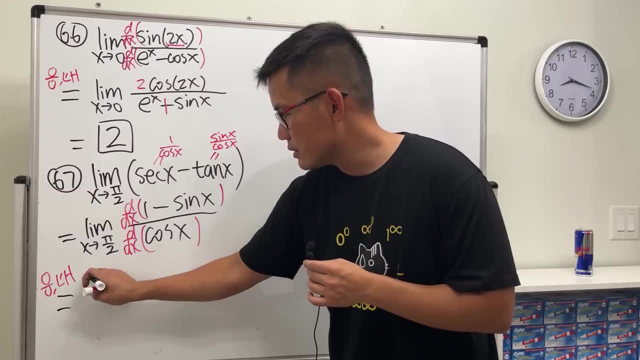 to mention that We do not have to use L'Hopital's rule if you don't want to, But anyway, this is a 0 over 0 case. We're using L'Hopital's rule. So this is the limit as x approaching pi over. 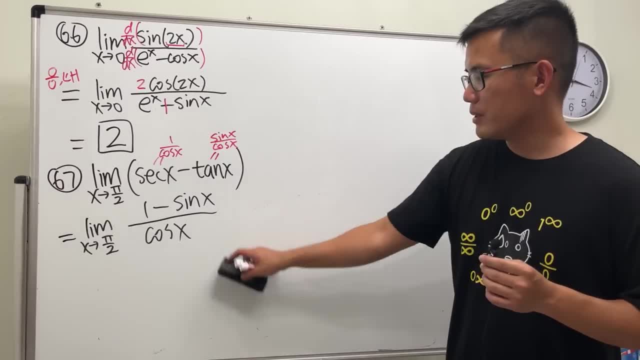 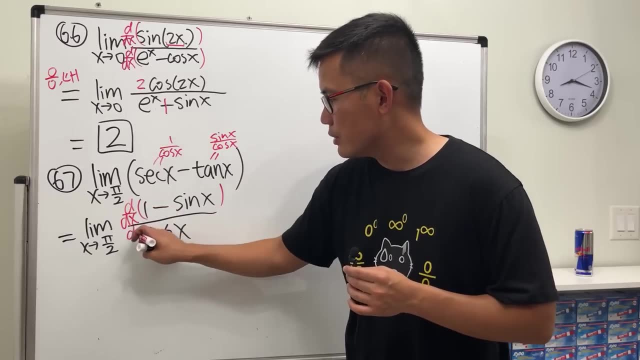 You can do it that way, But since this is the L'Hopital's rule category, so let's just use L'Hopital's rule. Just want to mention that we do not have to use L'Hopital's rule if you don't want to. 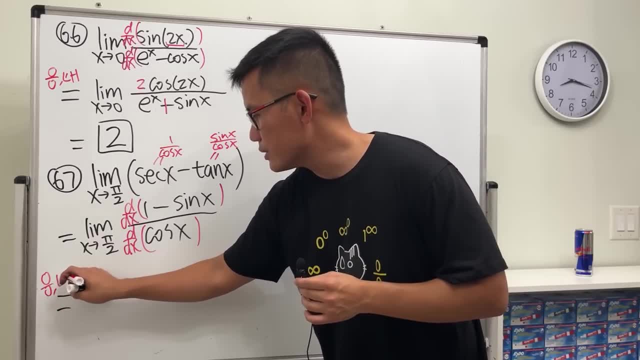 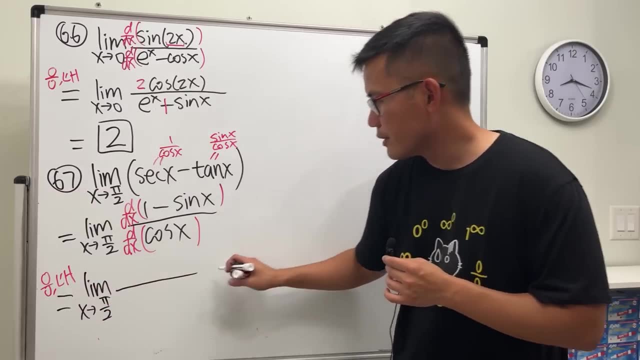 But anyway, this is a 0 over 0 case. We're using L'Hopital's rule, So this is the limit as x approaching pi over 2.. Derivative 1 is 0.. Derivative negative sine is negative cosine. 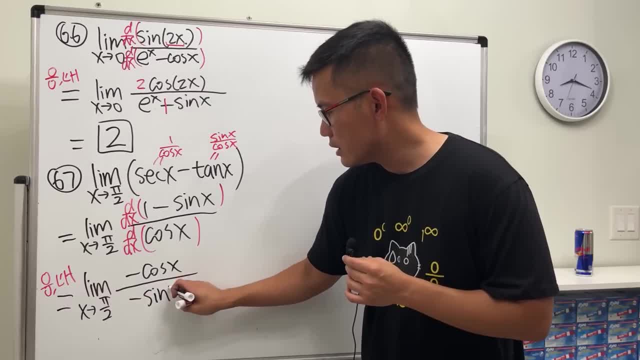 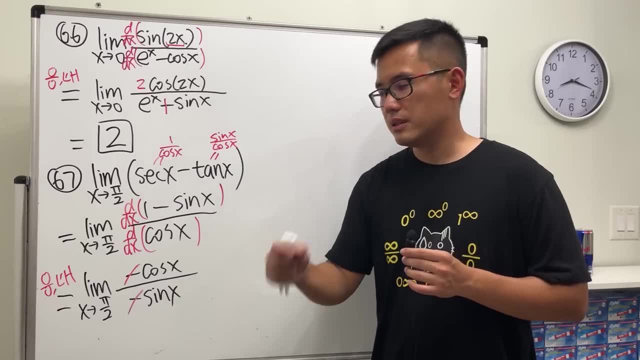 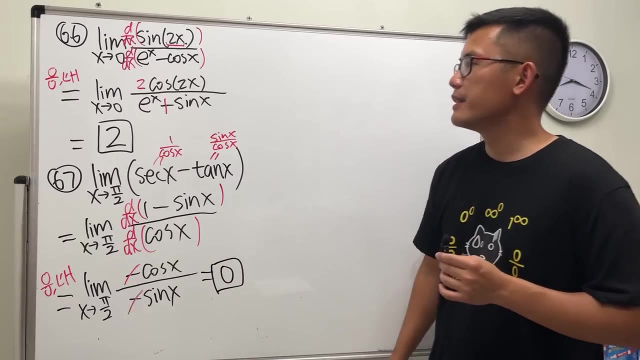 Derivative of cosine x is negative sine. So cancel Pi over 2.. Plug into cosines 0.. Sine of pi over 2 is 1.. 0 over 1 is 0.. Very cool, Alright. Oh, this is what I like. 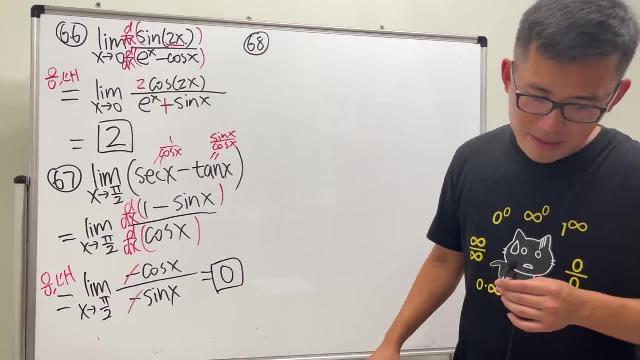 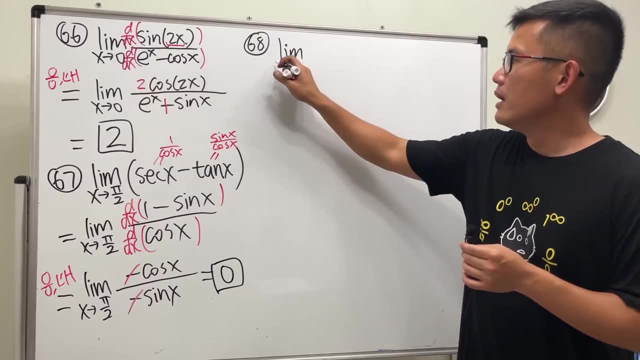 I can do multiple equations on the same board So I don't have to erase, erase, erase. Okay, number 68.. Another big one. Well. finally, x is approaching 1.. Well, that was an interesting number too. 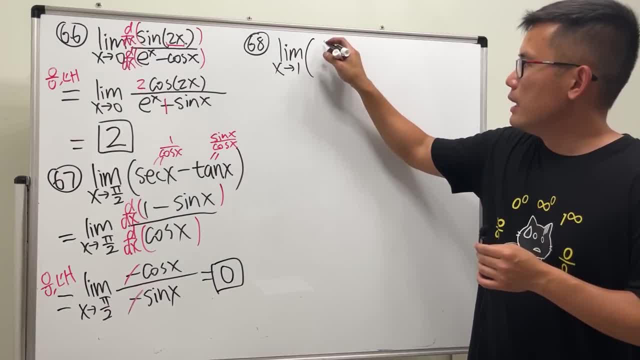 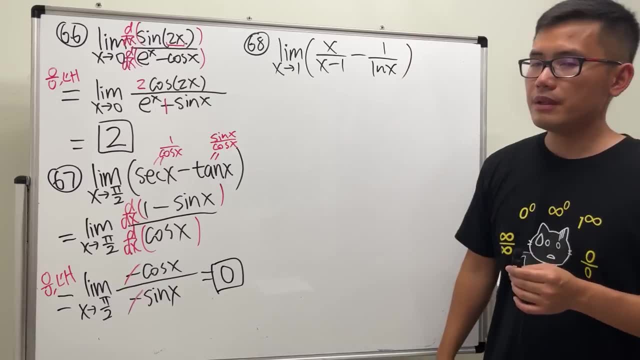 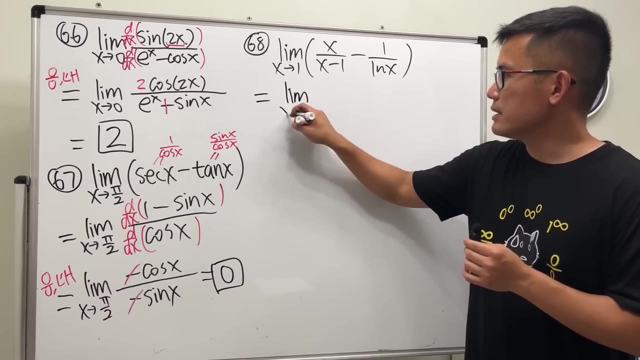 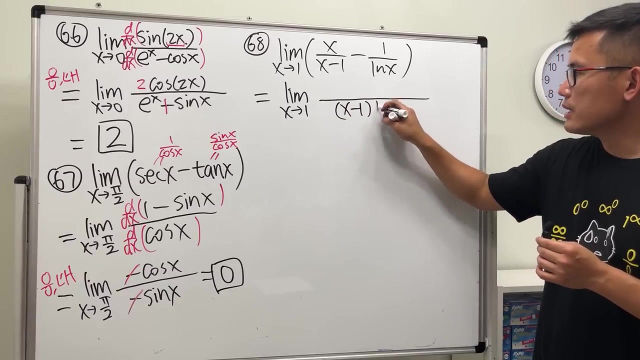 But anyway, x over x minus 1, and then minus 1 over Lnx. You know it, Combine the fractions before we continue. So number 68.. Here we go. Take the limit as x approaching 1.. This and that, on the bottom I will put it as x minus 1, parentheses times Lnx. 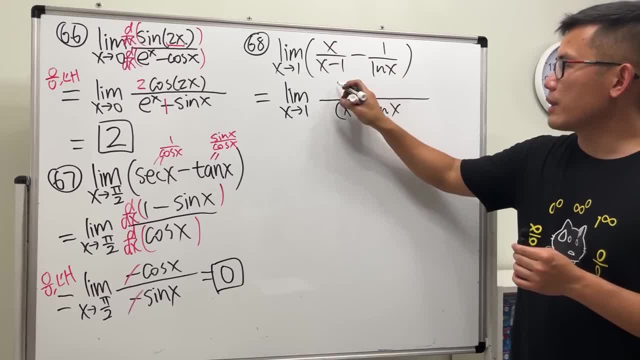 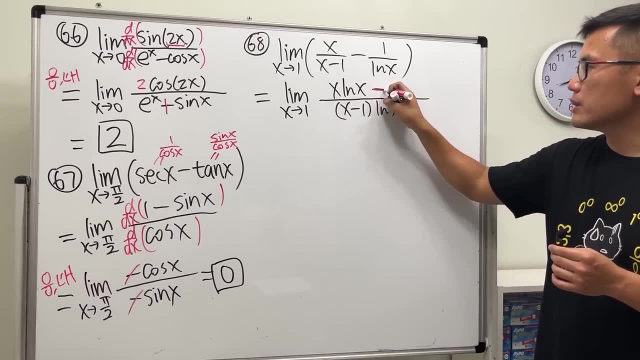 On the top, though I will do this: times that, right, x, times Lnx, And then minus this and that, which is just So I'm going to distribute. So it's minus, right, Minus x, Minus, minus become plus and then 1.. 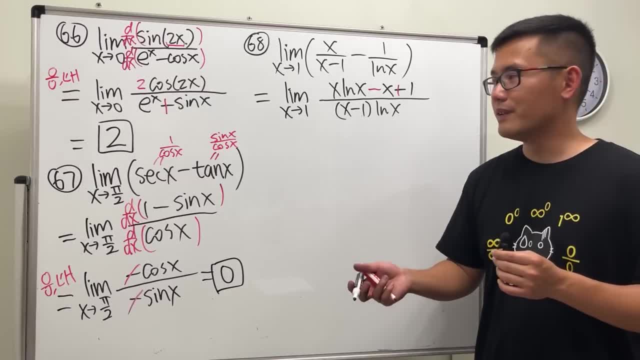 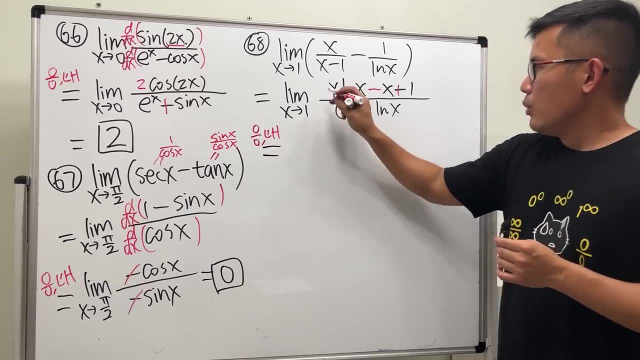 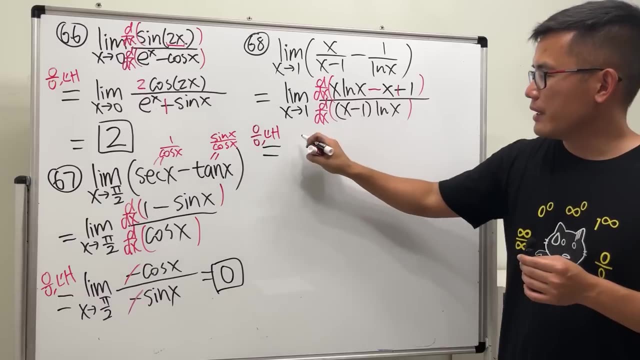 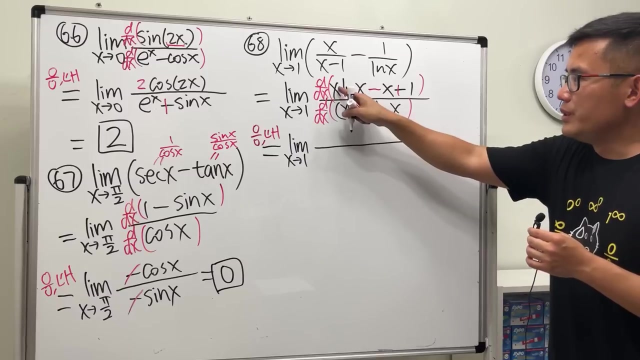 Alright, And then verify it, You get 0 over 0. So again, that's just the Lapito's rule. So the x- Okay, here is the limit as x approaching 1.. Okay, Product rule. here We need to keep the first function, which is x times the derivative of the second. 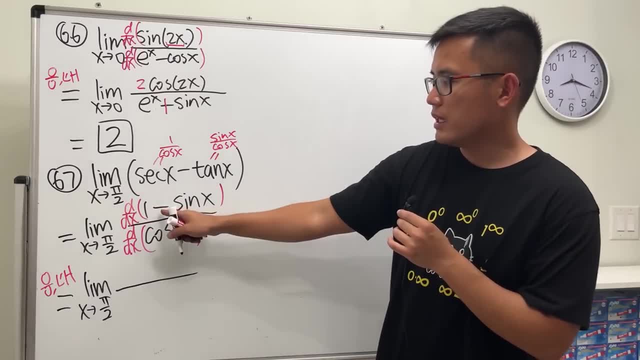 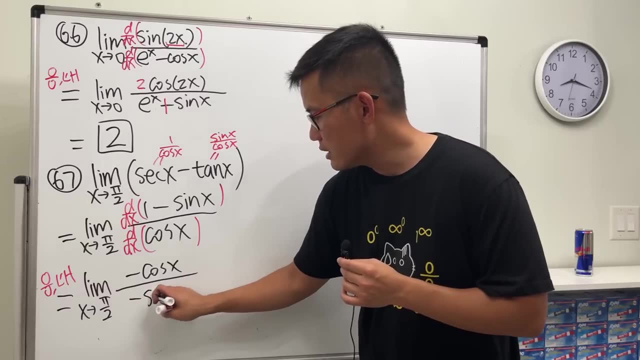 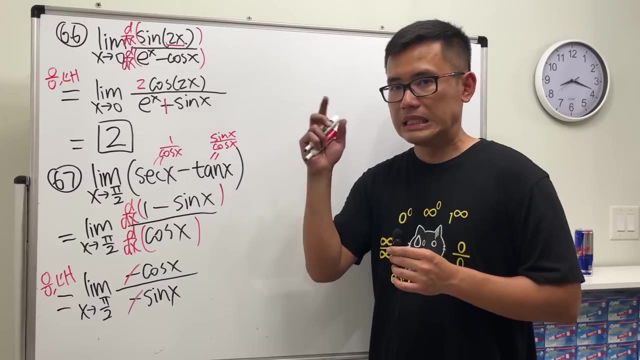 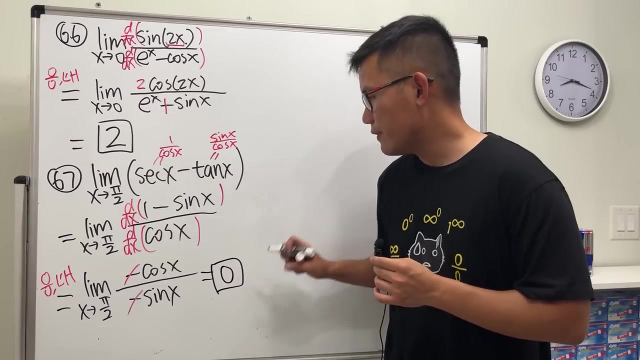 2.. The derivative 1 is 0.. The derivative negative sine is negative cosine. The derivative of cosine x is negative sine. So cancel Pi over 2.. Plug into cosines 0.. Sine of pi over 2 is 1.. 0 over 1 is 0.. Very cool, All right Oh. 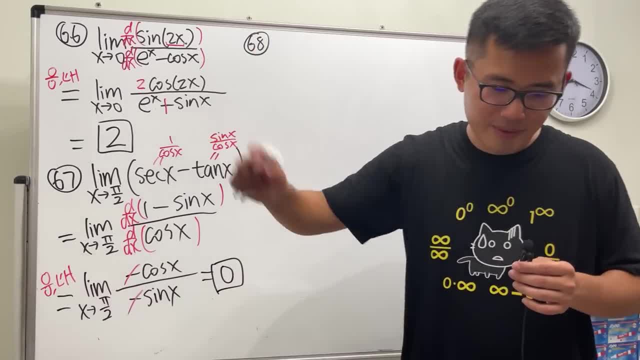 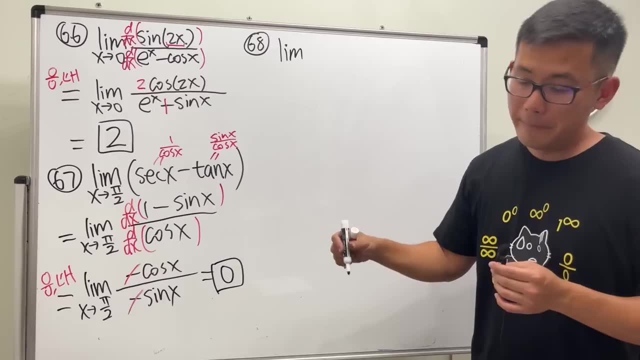 this is what I like. I can do multiple equations on the same board, So I don't have to erase, erase, erase. Okay, number 68.. Another big one, Oh, finally, x is approaching 1.. Well, that was an interesting number too, But anyway. 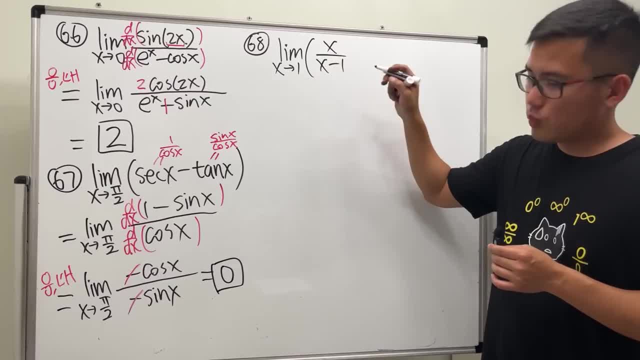 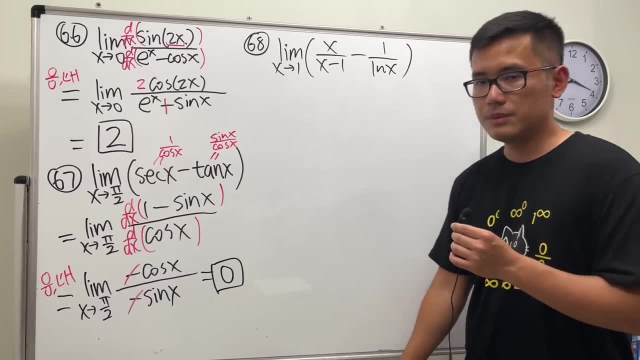 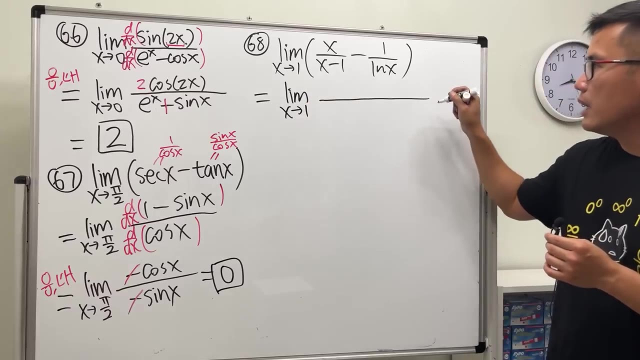 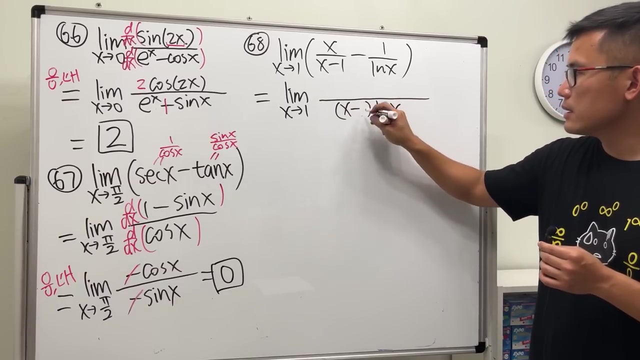 x over x minus 1, and then minus 1 over Lnx. You know it, Combine the fractions before we continue. So number 68.. Here we go. Take the limit as x approaching 1.. This and that. on the bottom I will put it as x minus 1, parentheses times Lnx. On the top though, 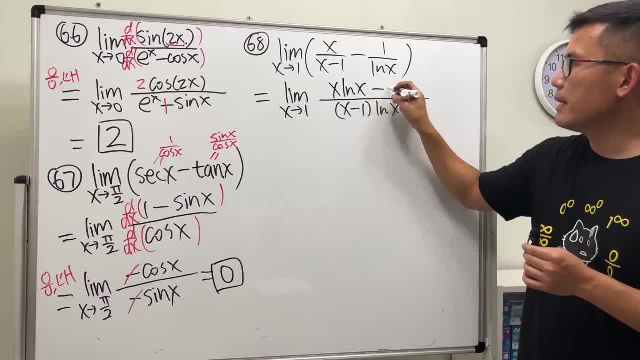 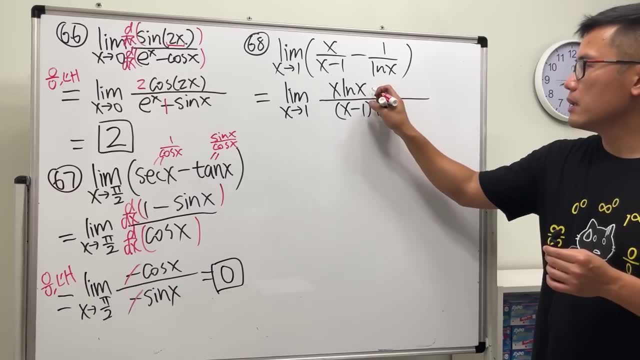 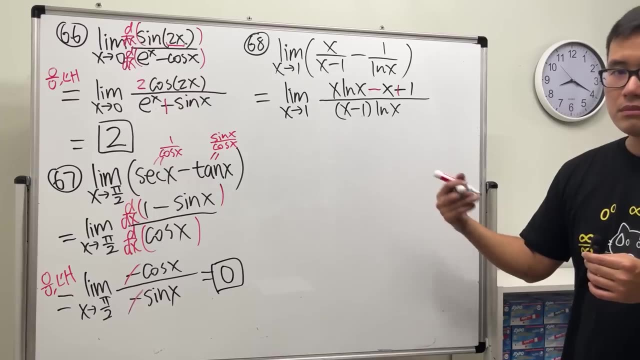 I will do this times that, right, So it's x times Lnx, And then minus This and that which is just, So I'm going to distribute. So it's minus, Minus, x, Minus, Minus, Become plus, And then 1.. All right, And then verify it, You get 0 over 0.. So again, 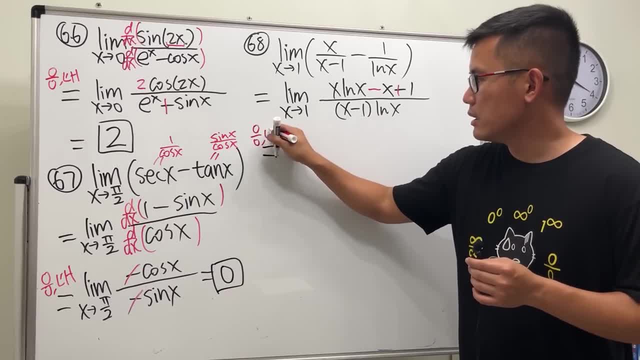 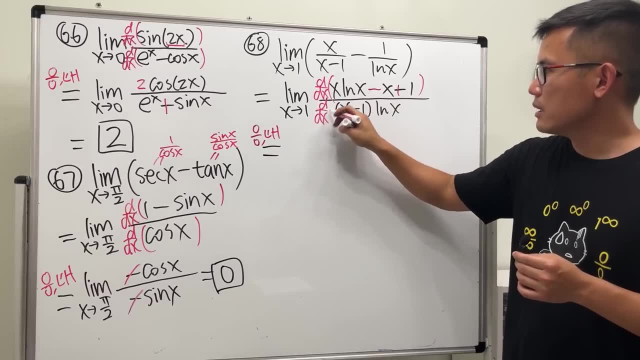 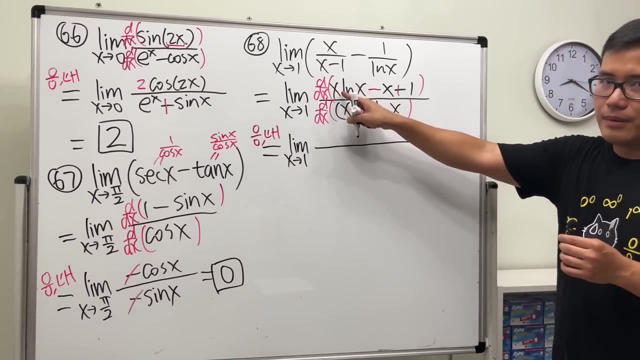 that's just the Lapito's rule. Wow, d dx. Okay, Here is the limit as x approaching 1.. Okay, Product rule: here We need to keep the first function, which is x times the derivative of the second And derivative of. 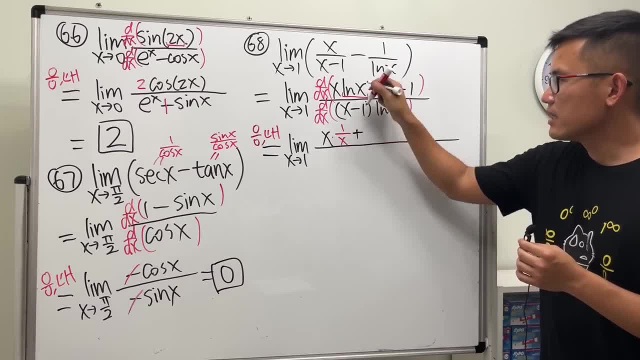 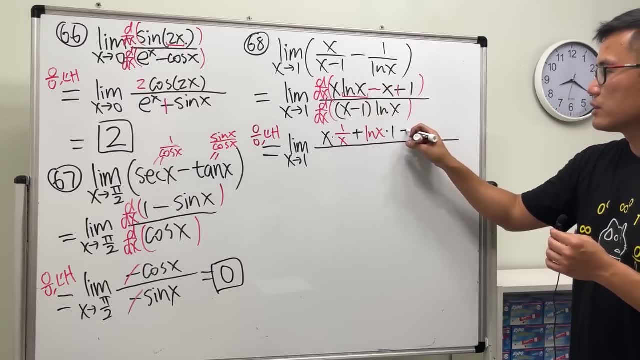 Lnx is 1 over x. And then we add the second function, which is Lnx times the derivative of the first, which is 1.. Continue: Derivative of minus x is just minus 1.. Derivative of 1 is 0. Done, Continue, Right here. 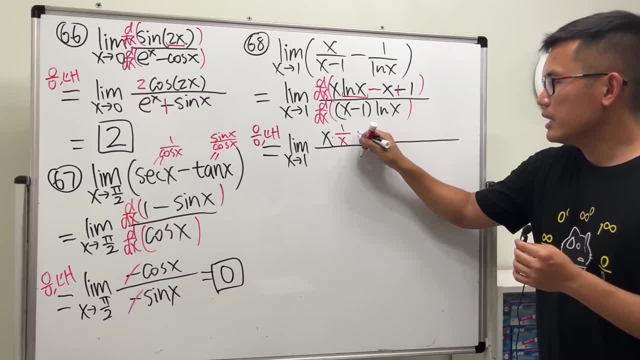 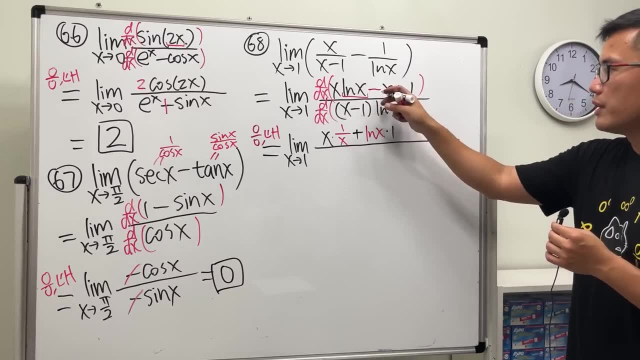 And derivative of Lnx is 1 over x. And then we add the second function, which is Lnx times the derivative of the first, which is 1.. Continue, The derivative of minus x is just minus 1.. The derivative of 1 is 0.. 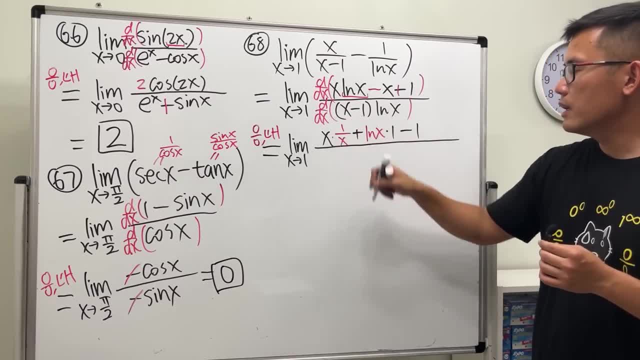 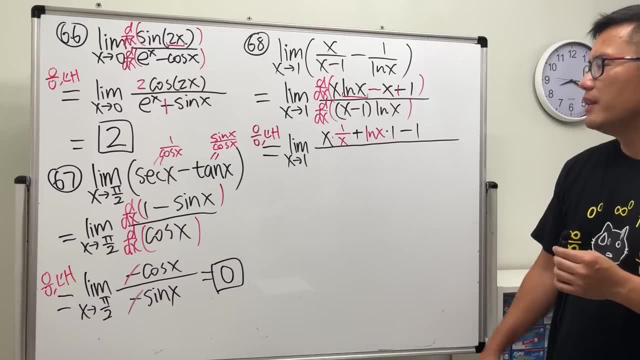 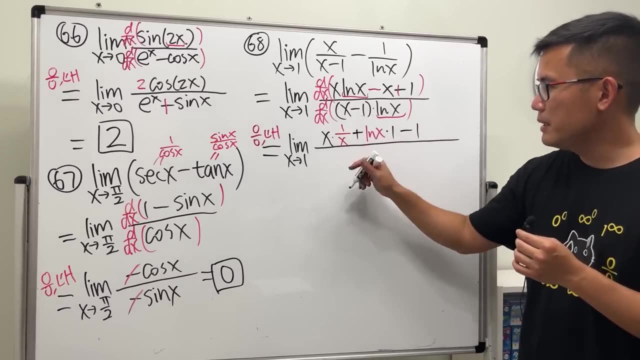 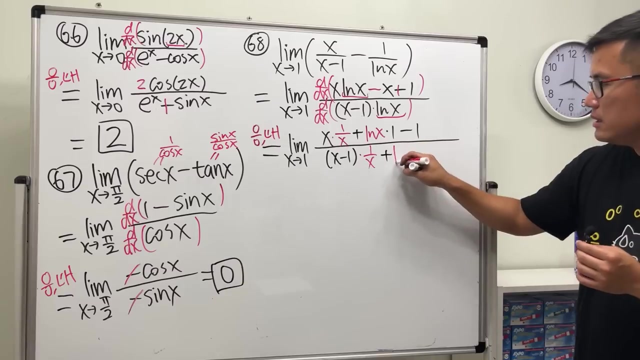 Done. Continue right here. Should we distribute it? Nah, let's just do it like this: Keep this as the first function and this as the second function. So I'm going to keep it as x minus 1 times the derivative of that, plus the Lnx times. 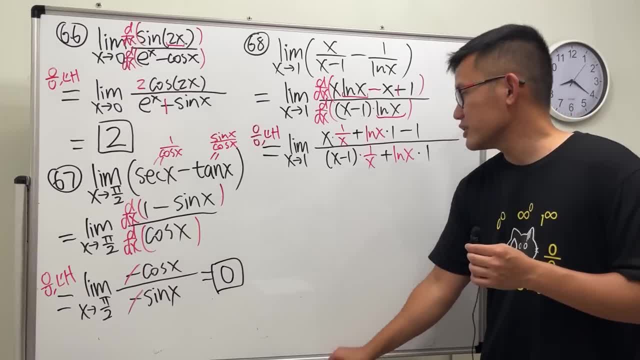 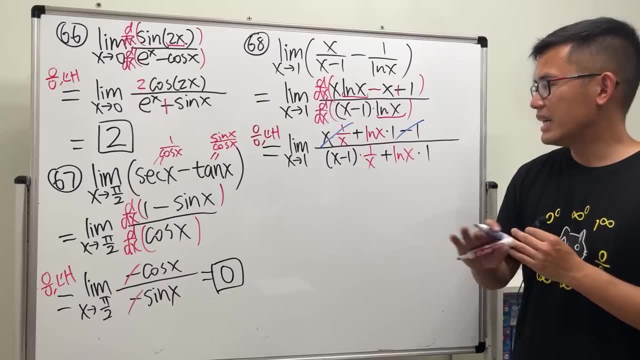 the derivative of that. Okay, Oh my god, Check this out. x over x is 1.. 1 minus 1 is 0. So, in fact, this and that cancel out completely Perfect. Here, though, we can distribute it. 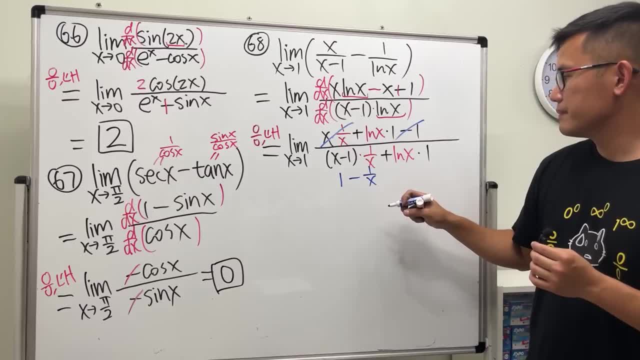 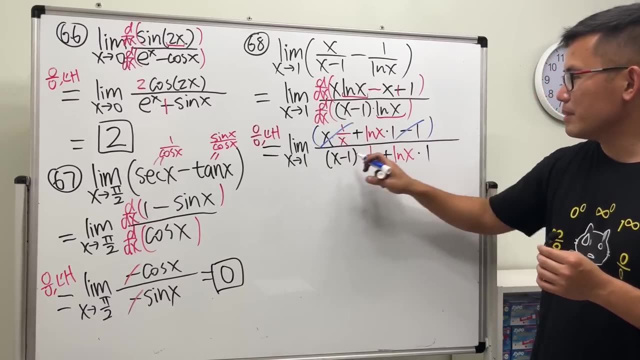 We get 1 minus 1 over x. That's still going to give us 0 over 0.. Oh, my goodness Right. So perhaps I'm not going to distribute it, because it doesn't do a single function If I distribute it. I'm just going to multiply the top and bottom by x so that we can get. 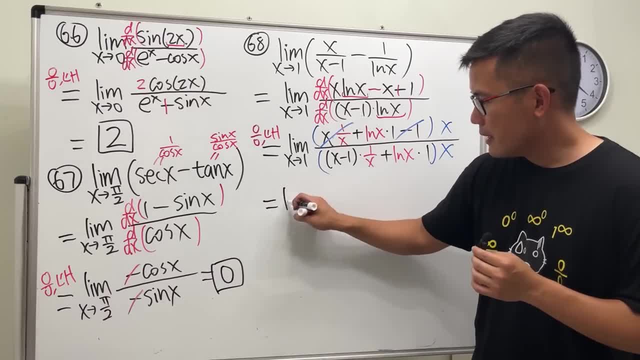 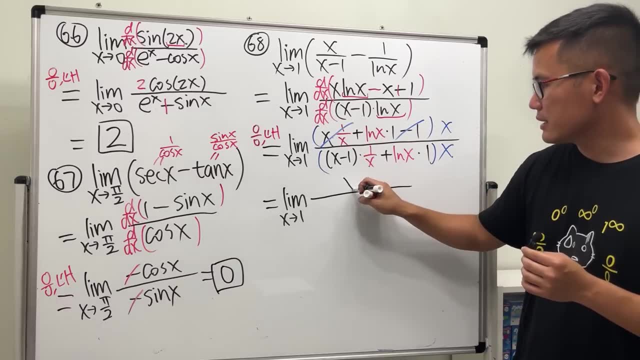 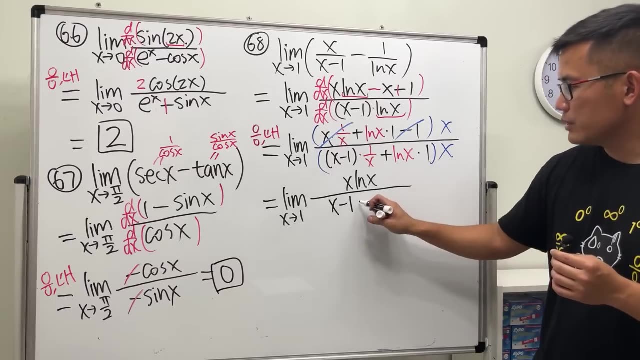 rid of that little x for the complex fraction case. So here we have the limit as x approaching 1.. This times that is just x times Lnx. Then this times that they cancel, which is just x minus 1.. And then this times that which is plus x, Lnx. 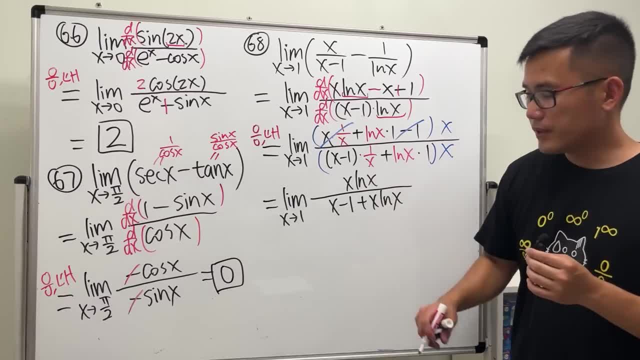 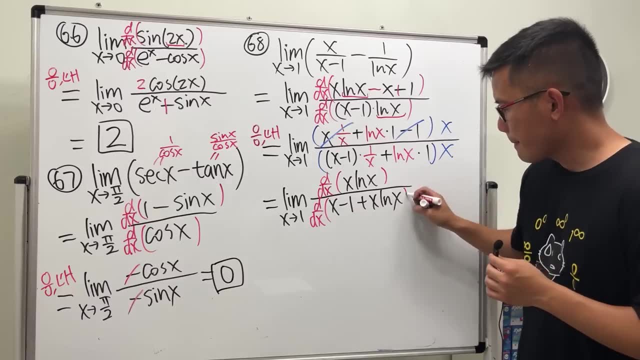 Okay, So we get 1 minus 1 over x. Yes, it's 0 over 0, but we can use Lapitov's rule again: Do this, Do that, So 0 over 0 Lh. 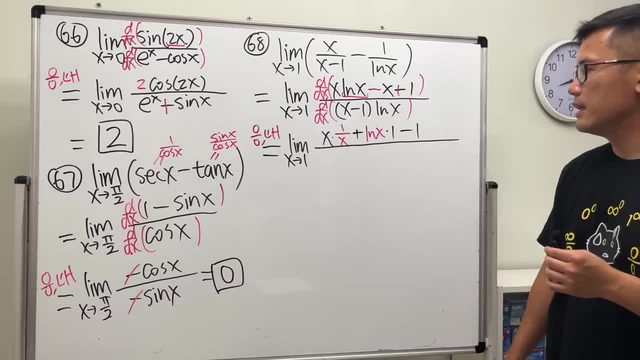 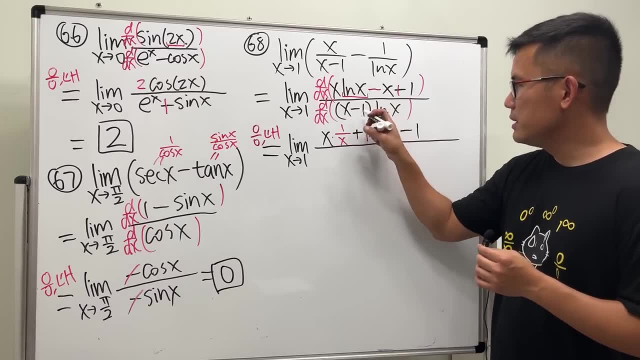 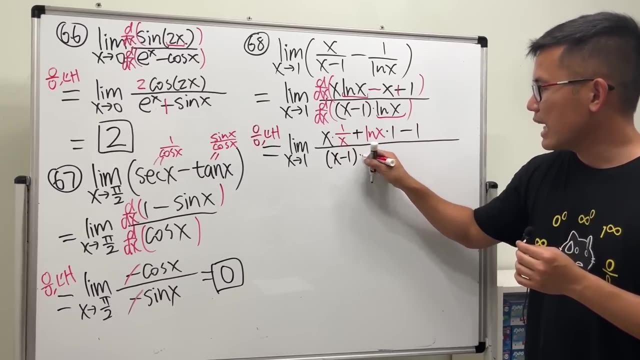 Okay, Now I just got to make sure. Should we distribute it? Nah, let's just do it like this: Keep this as the first function and this is the second function. So I'm going to keep it as x minus 1 times the derivative of that, plus the Lnx times. 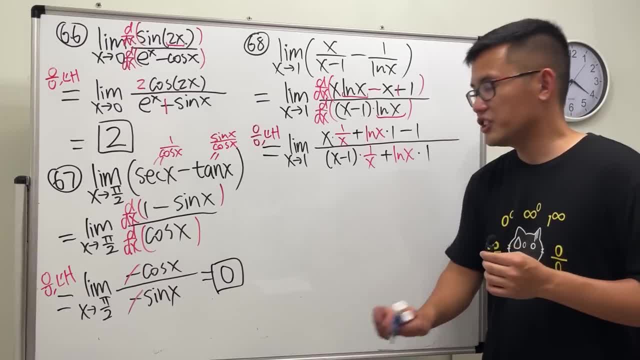 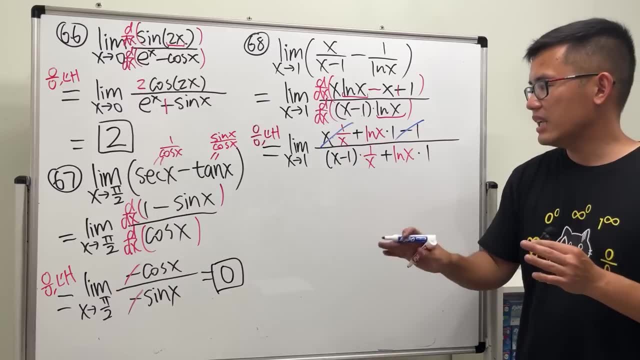 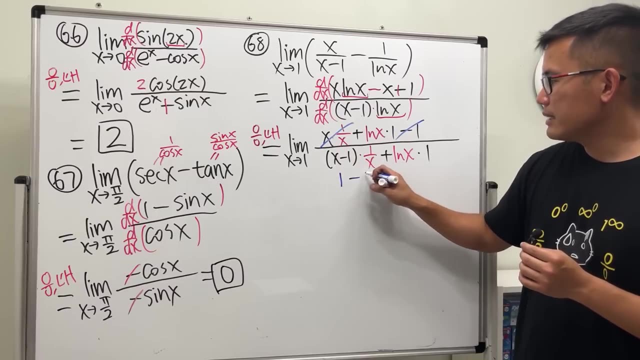 the derivative of that. Okay, Oh, my god, Check this out. x over x is 1, 1 minus 1 is 0. so in fact, this and that cancel out completely perfect. here, though we can distribute it, we get 1 minus 1 over X. that's still going to. 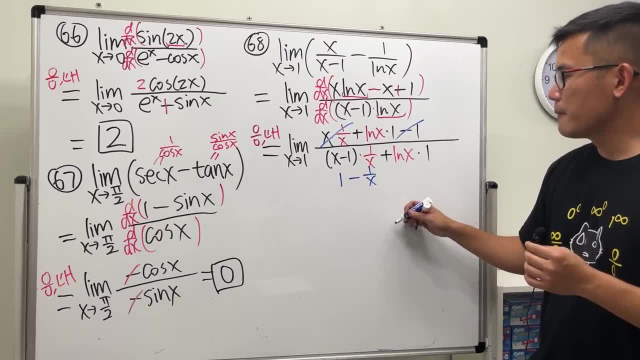 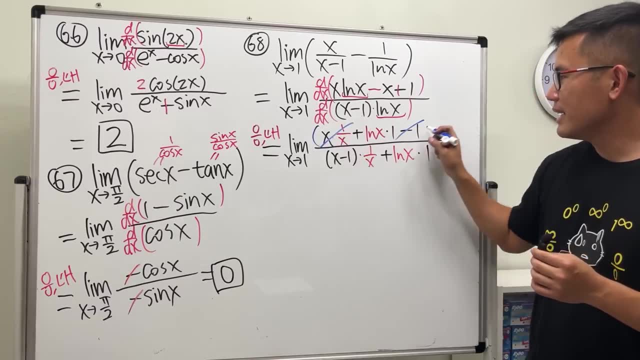 give us 0 over 0. oh, my goodness right. so perhaps I'm not going to distribute it because it doesn't do us any good. or if I distribute, I'm just going to multiply the top and bottom by X, so we can carry off that little X for the complex. 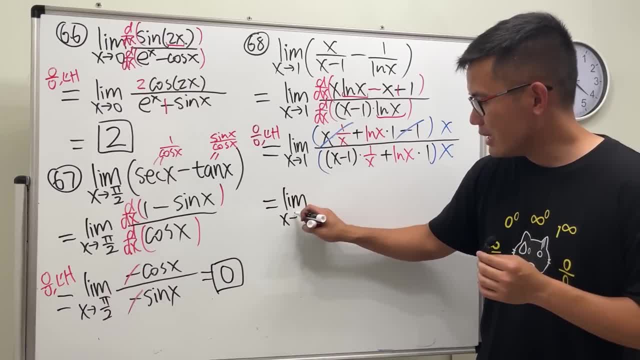 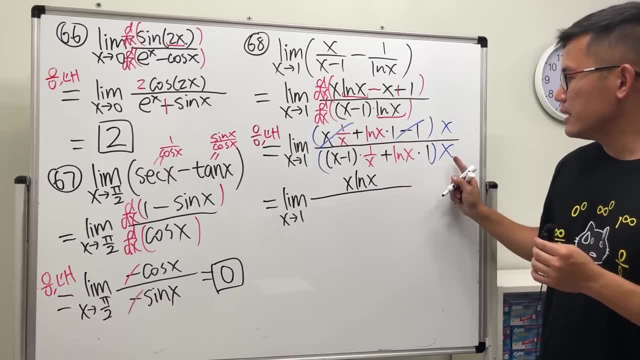 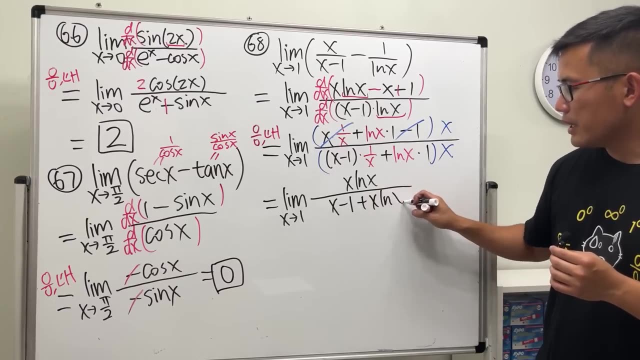 fraction case. so here we have the limit as X approaching 1, this times that it's just X, times L and X. then this times that they cancel, which is just X minus 1, and then this times that which is plus X, L and X. yes, it's 0 over 0, but we can. 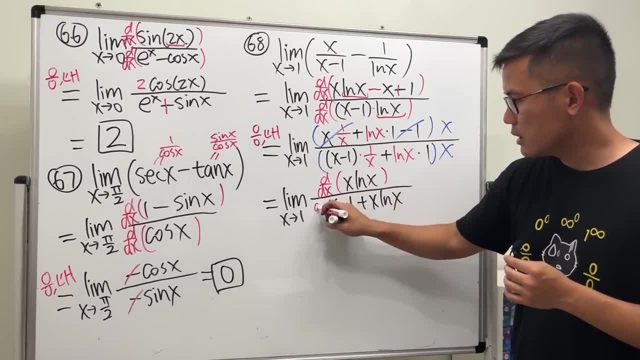 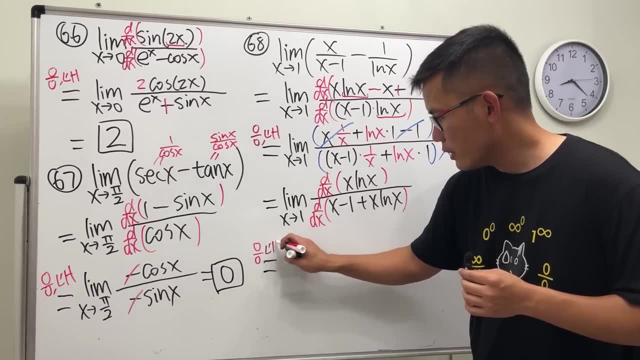 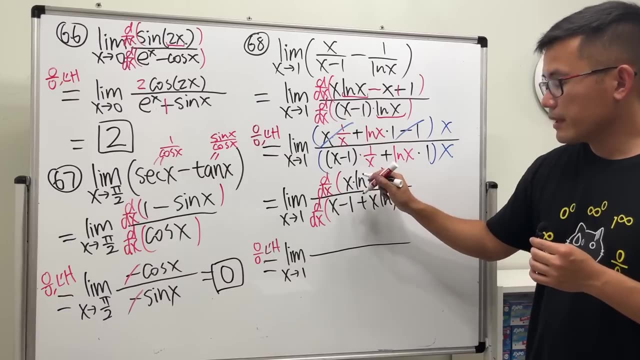 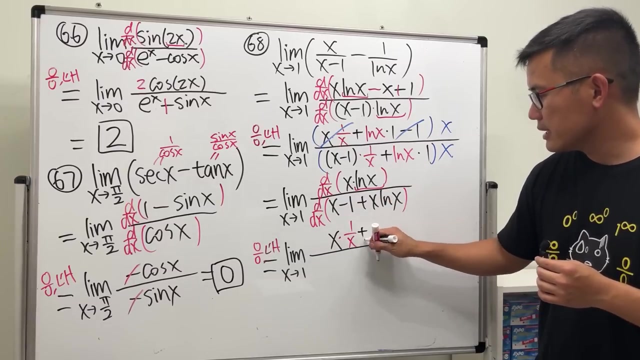 use Lapitov's rule again. do this, do that. so 0 over 0, L, H- this is the limit as X approaching 1. okay, Poitard rule in action: keep the first function, which is X times the derivative of the second, plus the second function, which is L and X times the. 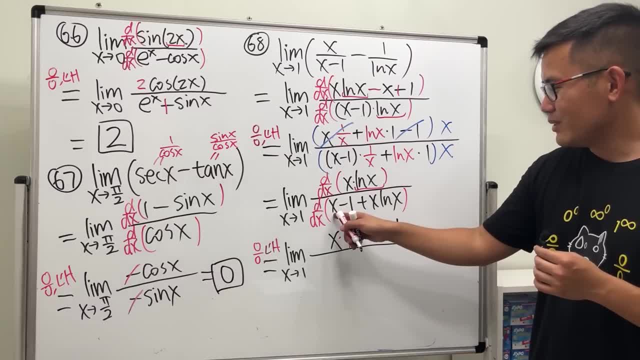 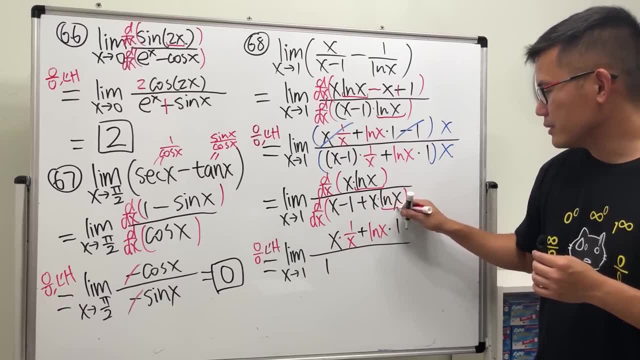 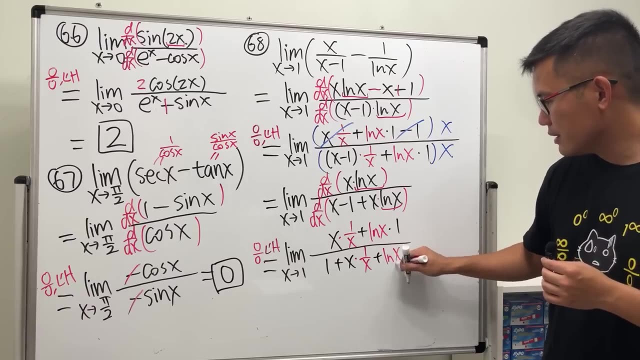 derivative of the first. now the derivative X is 1, the rudy of 1 is 0 minus 1 is 0. same thing here. quite a rule. plus first function times, detal of the second, plus the second function times the derivative first. oh my god. 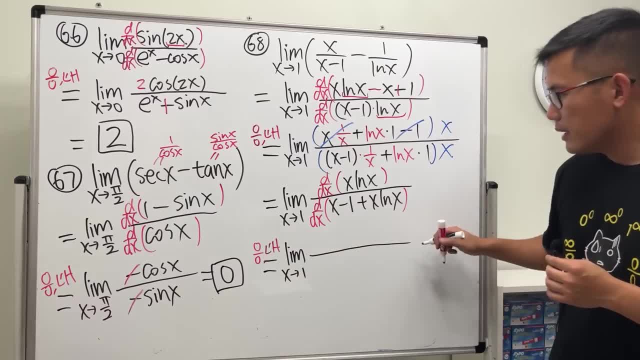 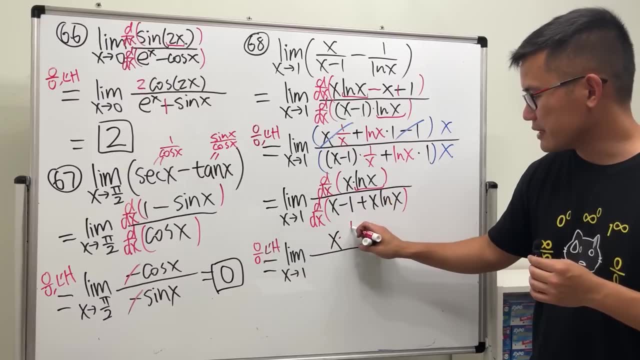 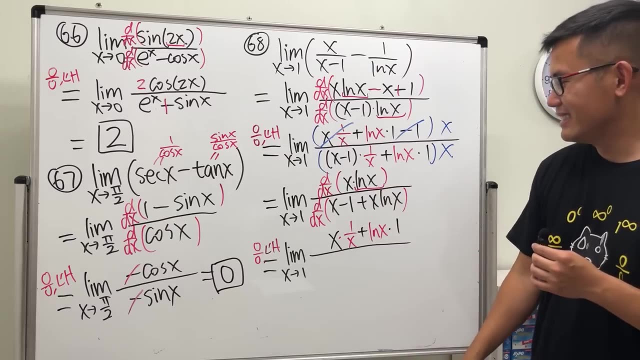 This is the limit as x approaching 1.. Okay, Poitard rule in action. Keep the first function, which is x times the derivative of the second, plus the second function, which is Lnx. This is 0 over 0 Lnx times the derivative of the second. 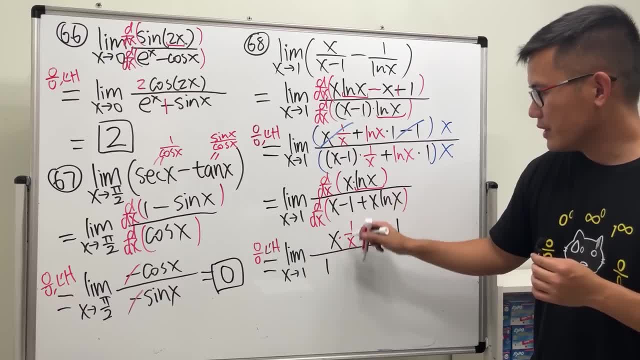 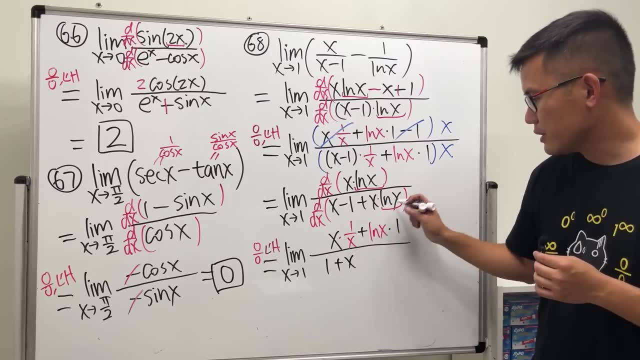 Now we have the first function, which is x plus x times the derivative of the second. Now the derivative of x is 1.. The derivative of 1 is 0, minus 1 is 0. Same thing here. 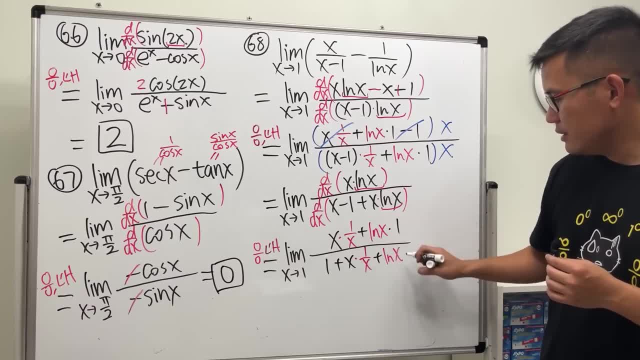 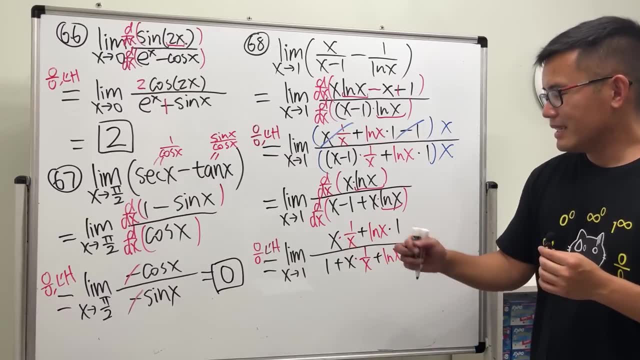 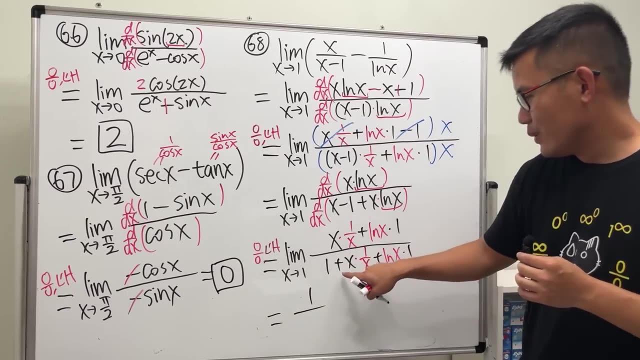 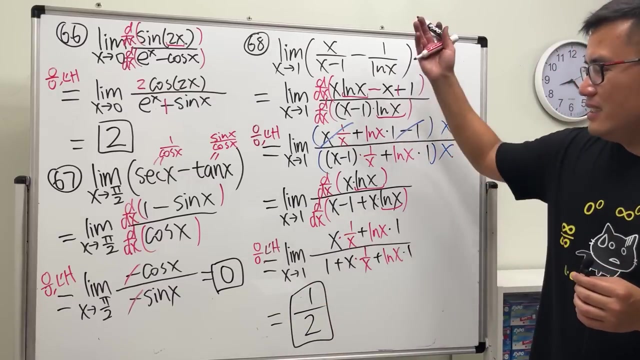 Poitard rule: Plus first function times the derivative of the second, plus the second function times the derivative of the first. Oh my god, Check this out. This is 1.. This is 1.. that's zero on the top. we have one. this is one. one plus one is two, ladies, and 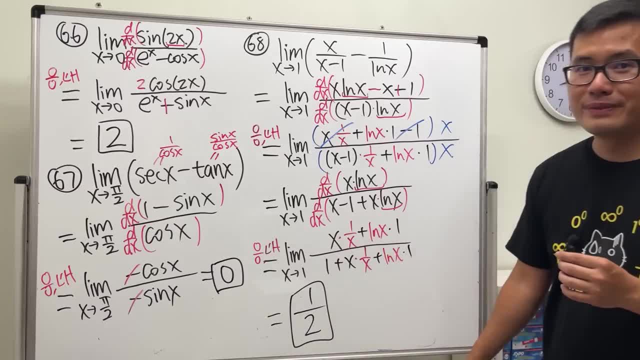 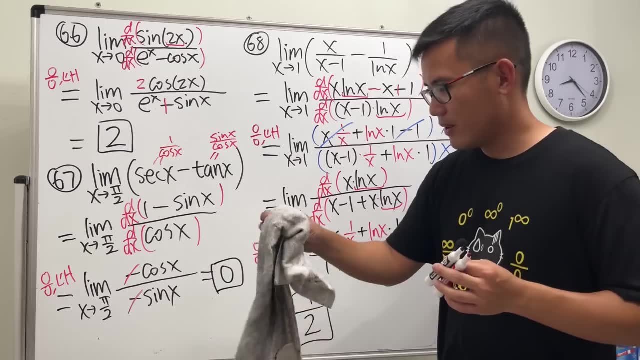 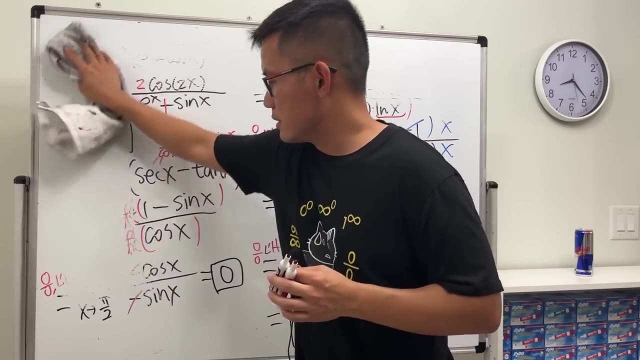 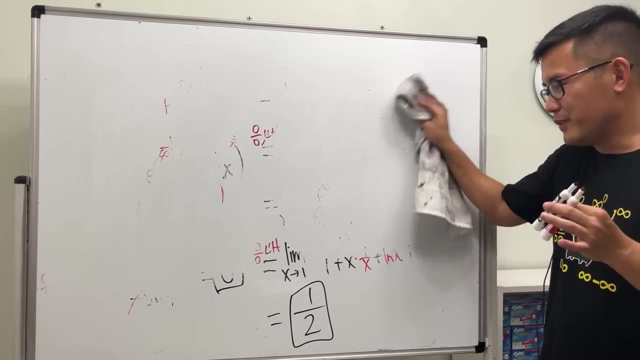 gentlemen, for all the work, we just get one half. yeah, all this work, we get one half. number 68: oh, my god, my hands are so dirty, so look at this. yeah, cool, you see, I'm doing so many questions for you guys, right? yeah, if you are taking 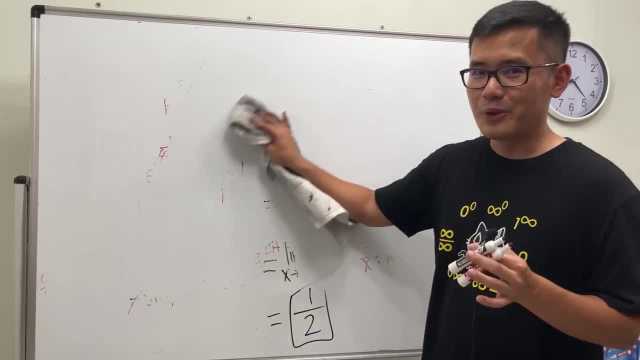 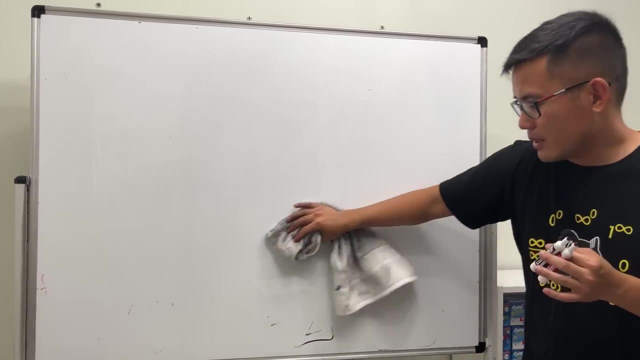 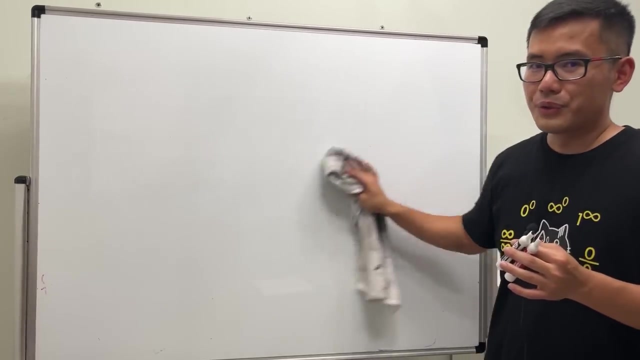 carbon for the very first time. how many questions are you practicing? that's the key, right, if you want to really learn calculus work- depending on if you really want to learn on material or if you just want to get over calculus practice. I'm doing this for you guys, with you guys. 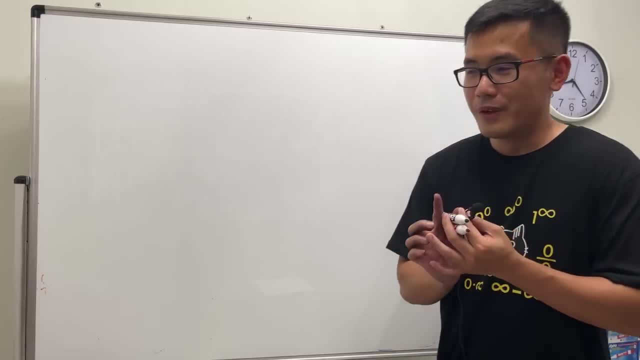 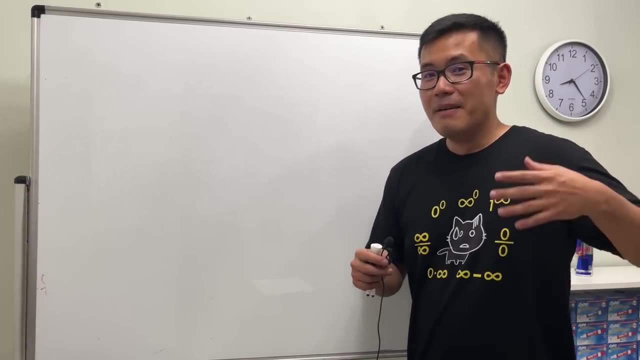 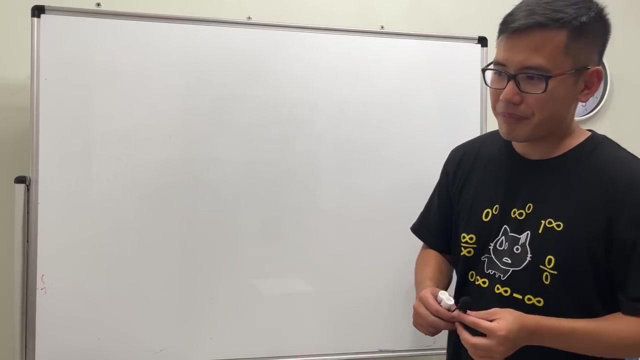 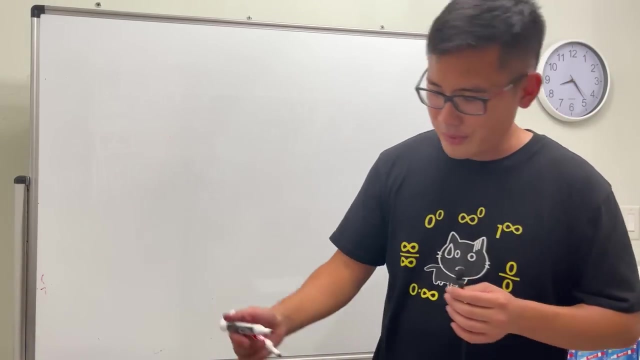 so maybe you are not like using, maybe you are not even though you're not, maybe you are just like studying for your calculus or math test in general. you are not really needing like this material. hopefully this can somehow motivate you in any way. anyway, this question number 69 and we have the limit as: 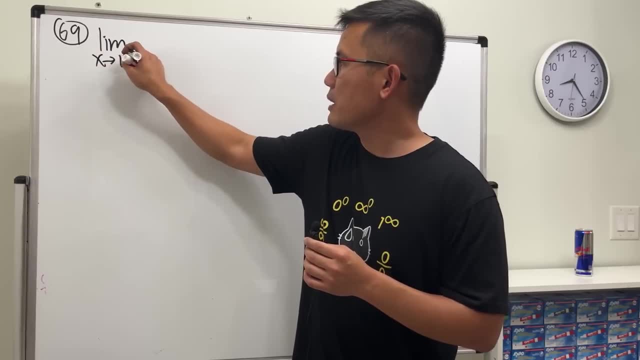 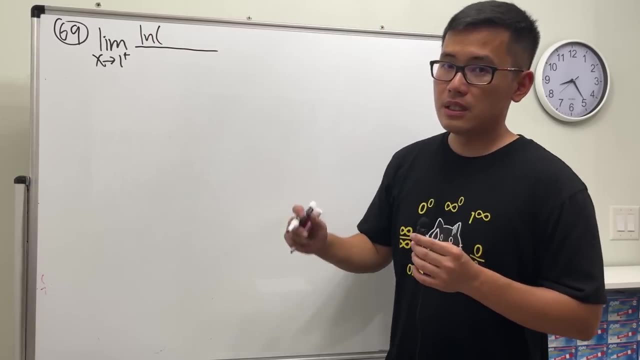 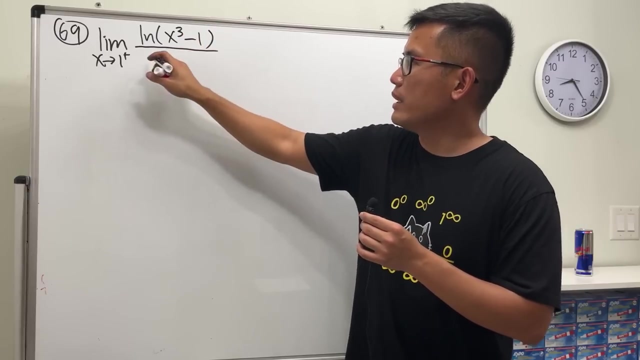 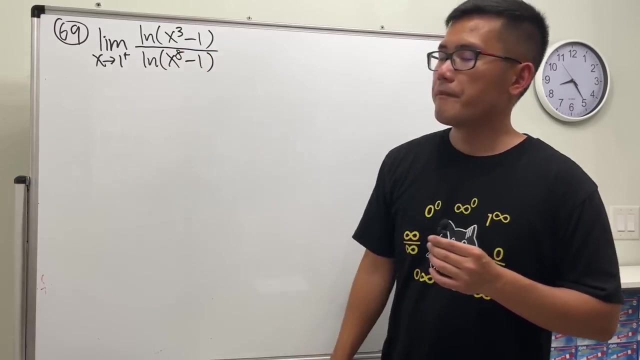 x approaching one plus and then we have natural log. I would like to tell you this is a very common test type of question. okay, LN on the top and then inside. here I picked X to the third power minus one. on the bottom I have LN of X to the eighth power minus one. very common, very popular calc 1 or calc 2. 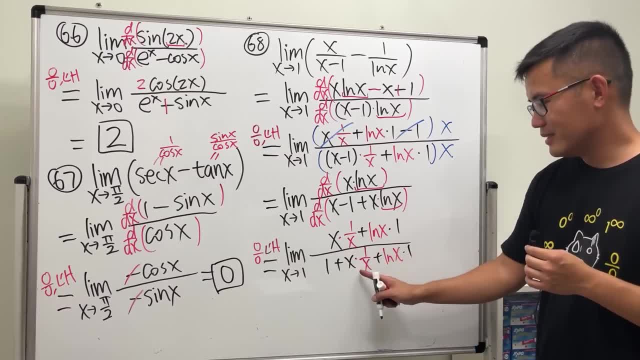 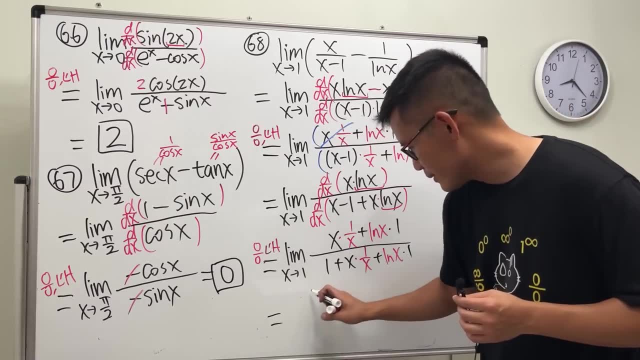 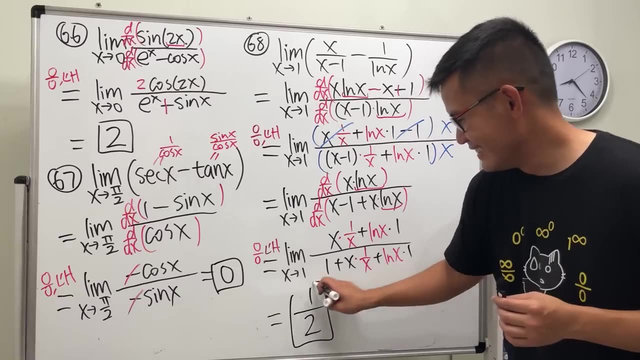 check this out. this is one. this is one. when X is approaching one. this is your rock dassero. on the top we have one. this is 1. One plus one is two. Ladies and gentlemen, for all the work, we just get one half. 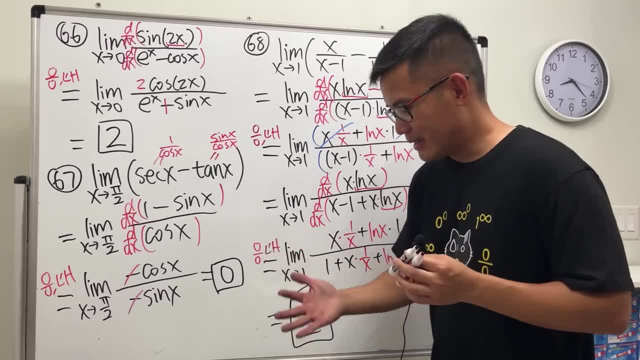 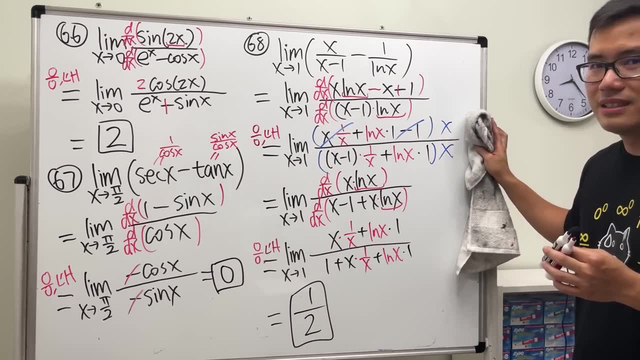 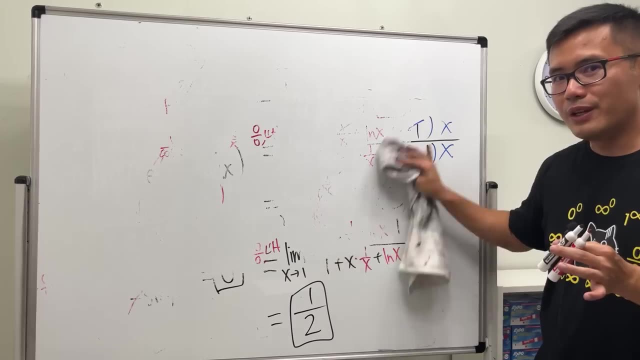 Yeah, all this work, we get one half. Wow, number 68.. Oh my god, my hands are so dirty. Look at this. Yeah, cool, You see I'm doing so many questions for you guys, right? Yeah, if you are taking Cal1 for the very first time, 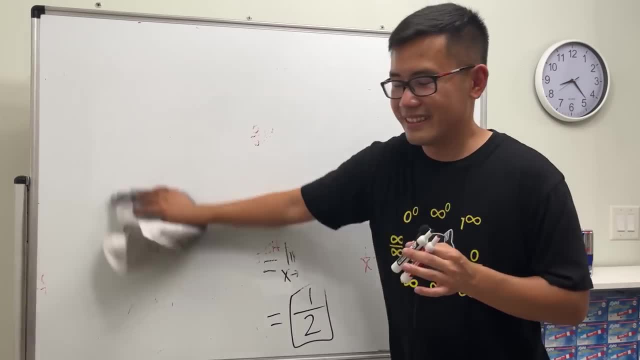 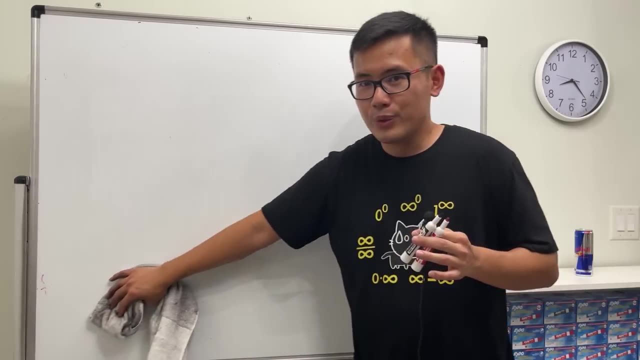 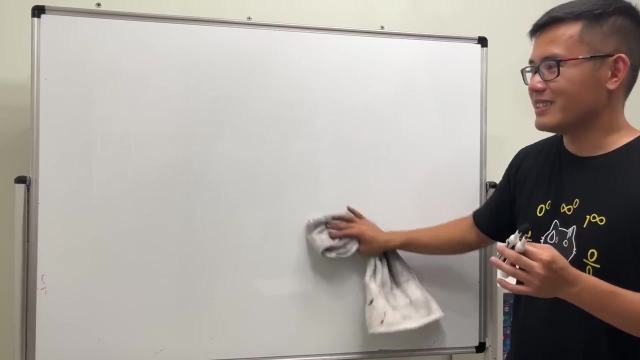 how many questions are you practicing? That's the key, right? If you want to really learn calculus or, depending on, if you really want to learn a material or if you just want to get over calculus practice. I'm doing this for you guys, with you guys, right. 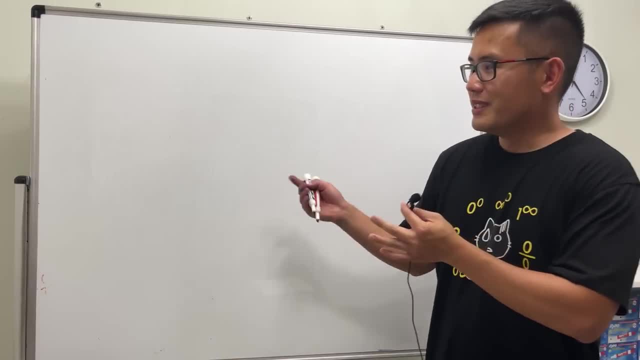 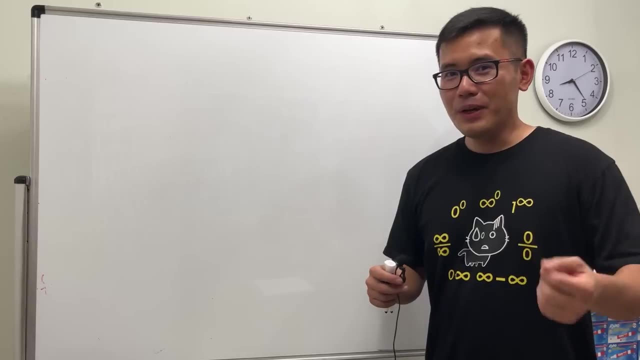 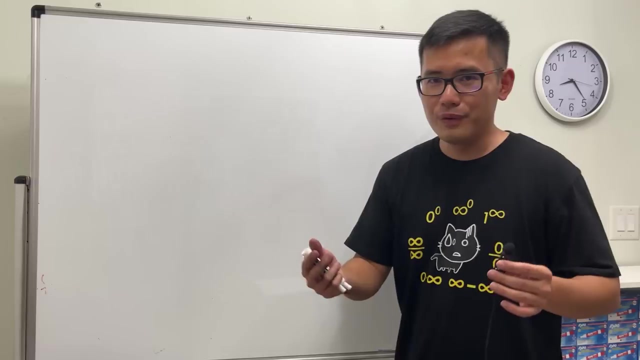 So maybe you are not like, maybe you are not even though you are not, maybe you are just like studying for your calculus or math test in general. you are not really needing like this material. Hopefully this can somehow motivate you in any way. 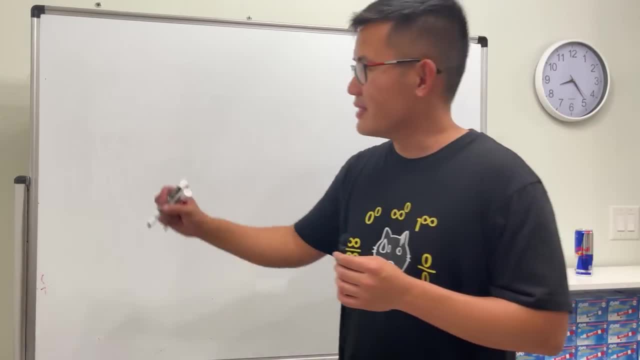 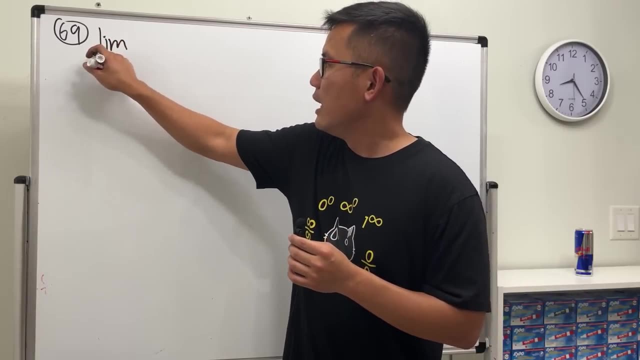 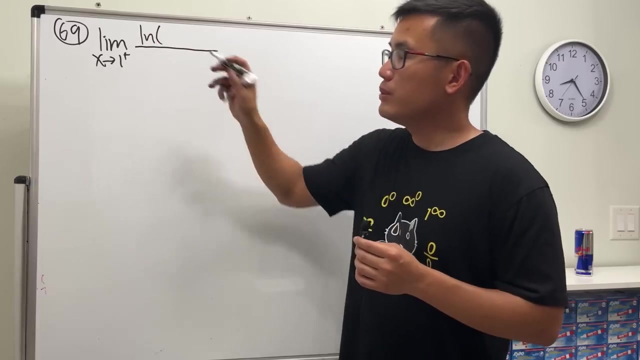 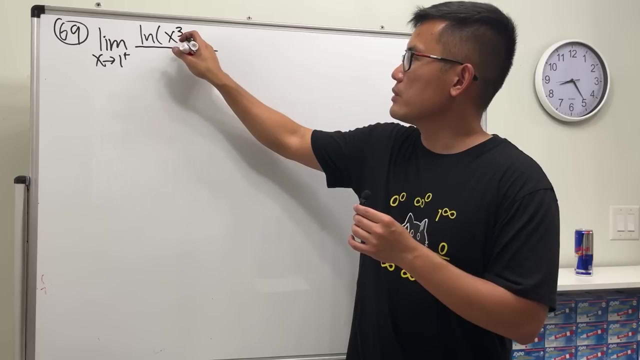 Anyway, this question Number 69, and we have the limit as x approaching one plus, and then we have natural log. I would like to tell you this is a very common test type of question. okay, Ln on the top and then inside. here I picked x to the third power minus one. 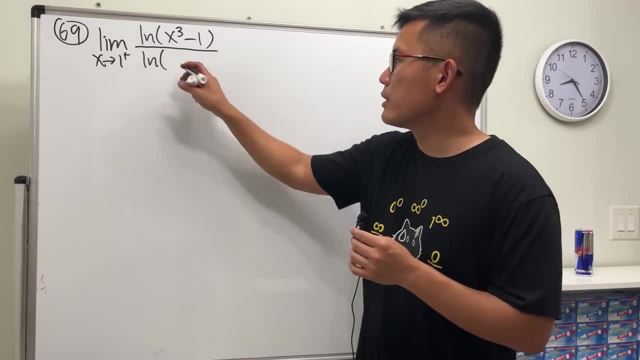 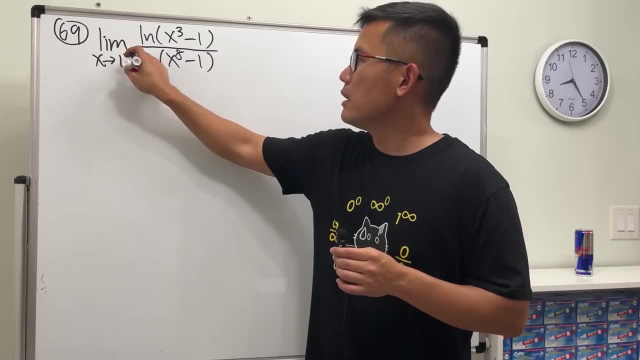 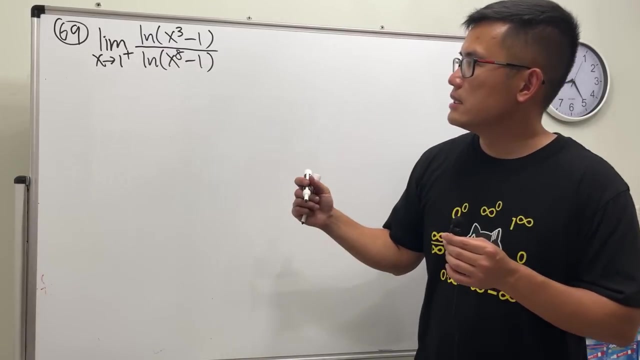 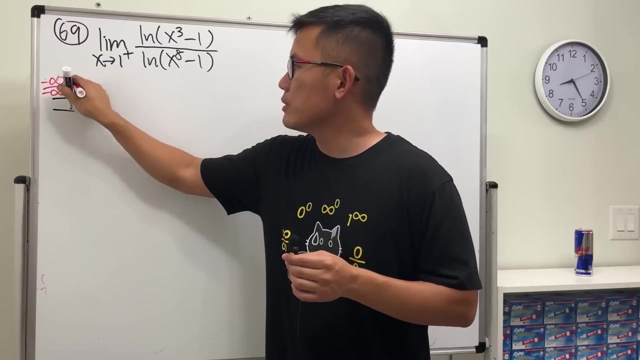 On the bottom I have Ln of x to the eighth power minus one Very common, very popular Cal1 or Cal2 test question. Okay, You will get negative infinity over infinity by, like, yeah, it just tells you you can do Lapito's rule. 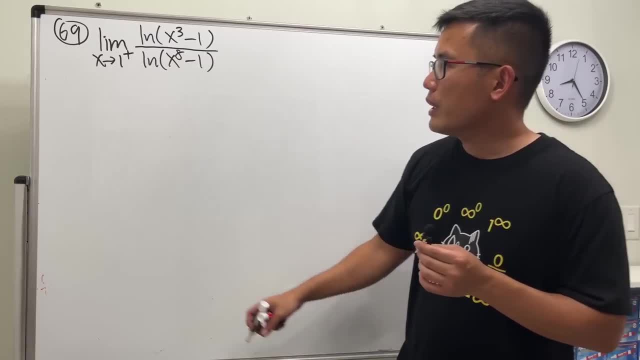 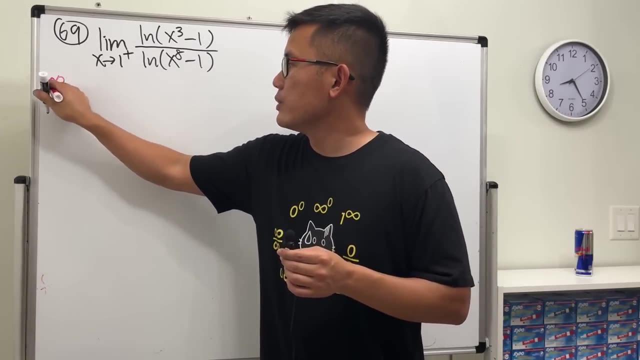 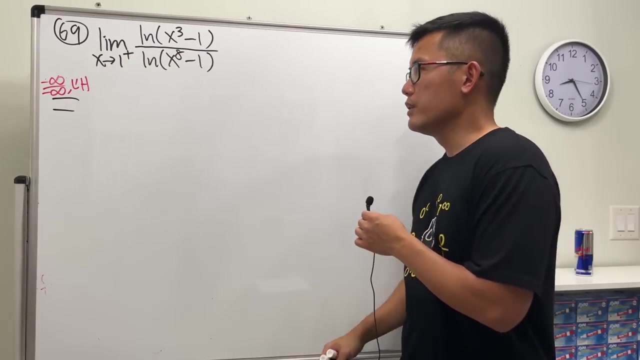 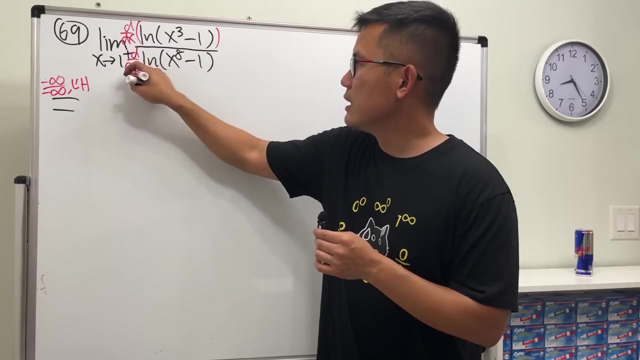 test question: okay, you will get negative infinity over infinity by like: yeah, it just tells you you can do a Lapito's rule, because we get LN of 0 plus. oh, no, 0 plus, that's why, anyway, the DX, DDX. okay, here we go. limit X approaching one. 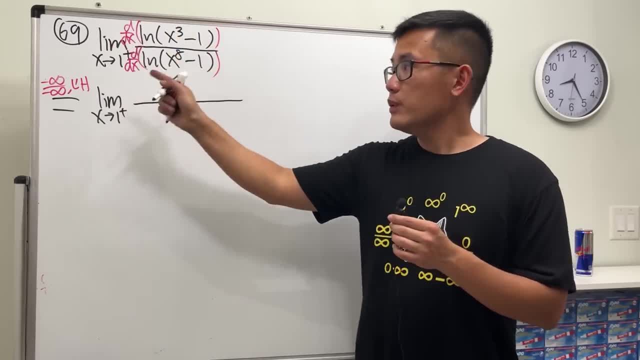 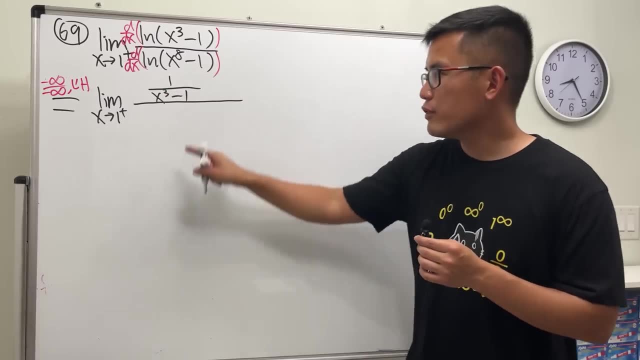 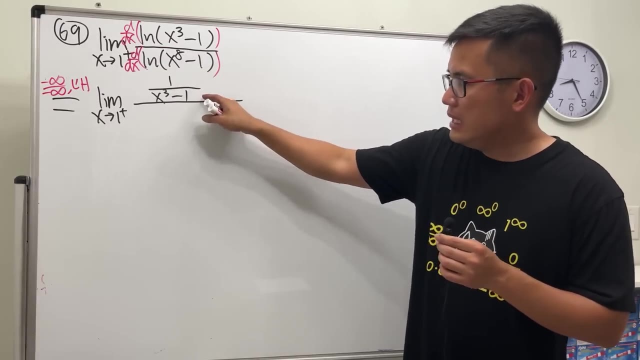 plus, when we differentiate LN we just put that on the bottom, so it's 1 over X to the third power minus 1. you don't have to multiply by LN of the base. technically you do. LN is log base E. when you have LN, E is just 1, so it doesn't. 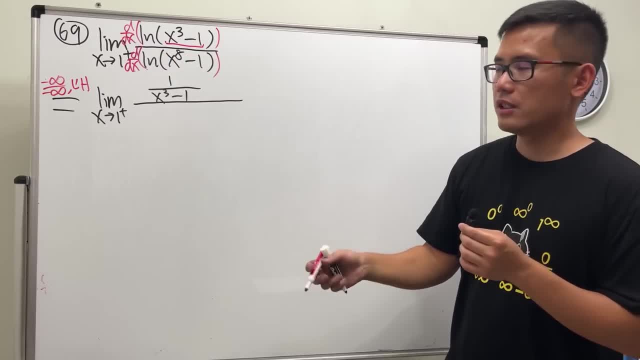 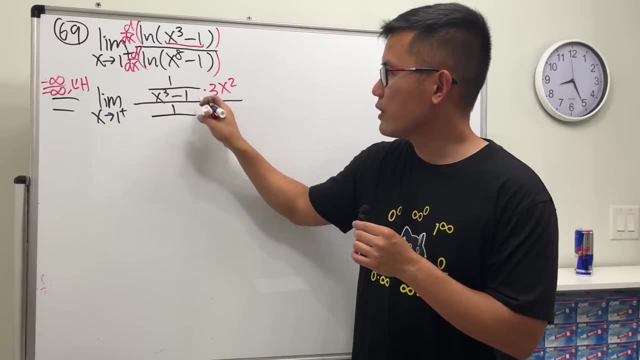 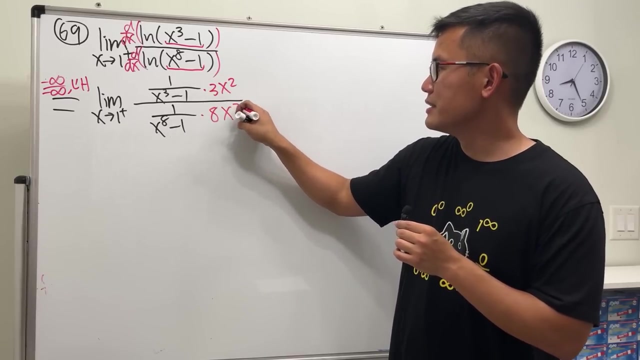 really matter anyway. multiply by the inside derivative, so that's the chain rule. so multiply by 3x square. do the same thing on the bottom. we get 1 over X to the eighth power, minus 1. and then multiply the derivative on the bottom, which is 8x to the seventh power. Wow, okay. so what we'll do next is- I'm just 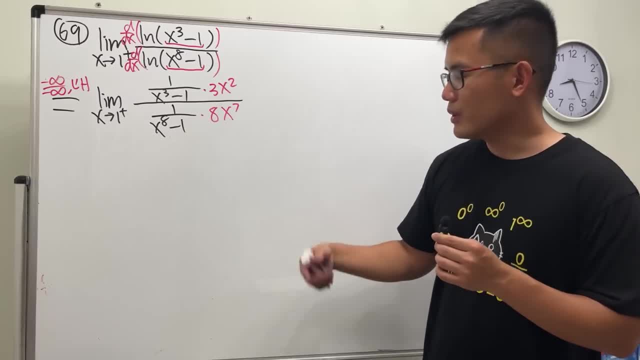 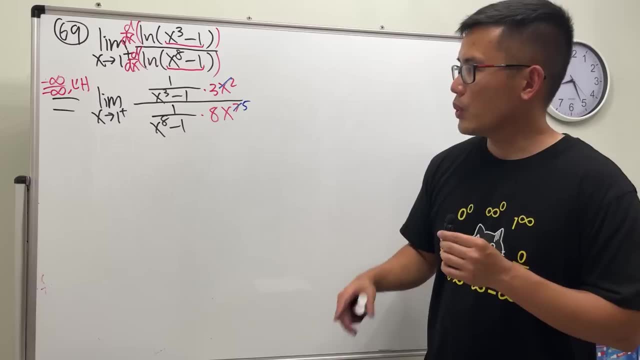 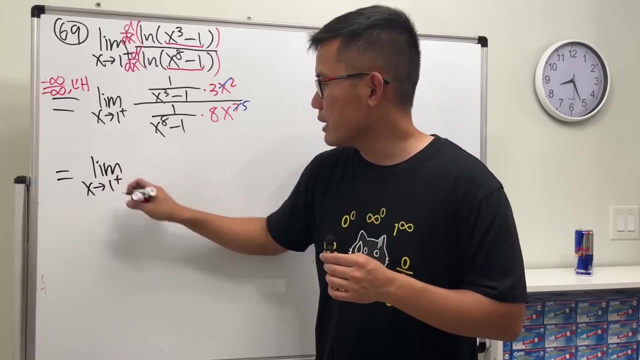 going to kind of: well, let's reduce this a little bit. yeah, this, and that would cancel, would become the fifth power, only cool. and then we are going to get the limit x approaching, one plus and uh, to make things more clear, i think i'm just going to do the stacy. 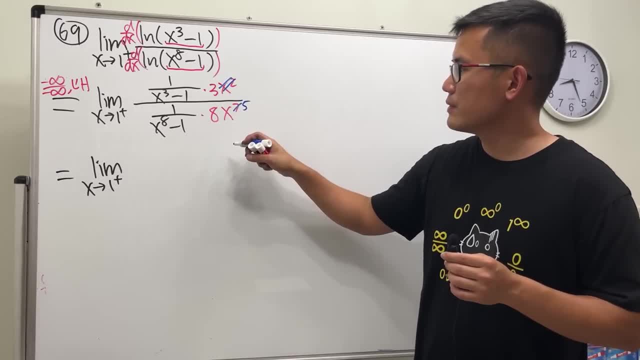 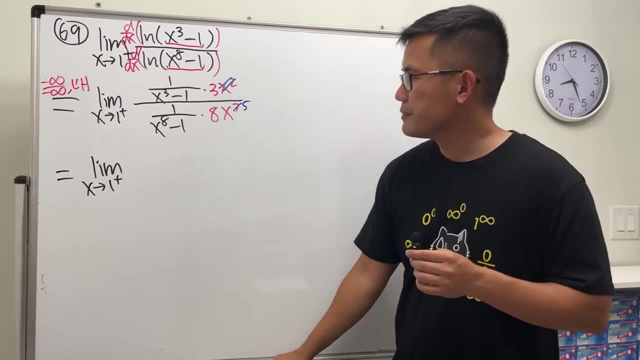 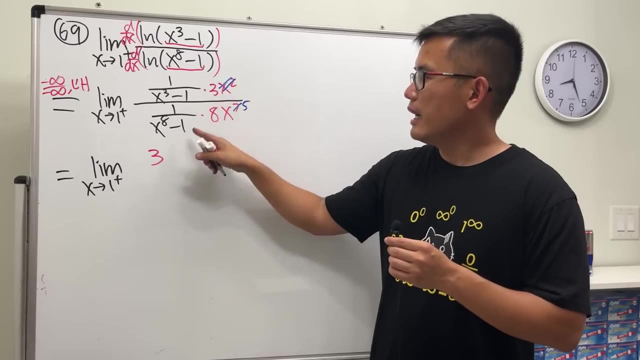 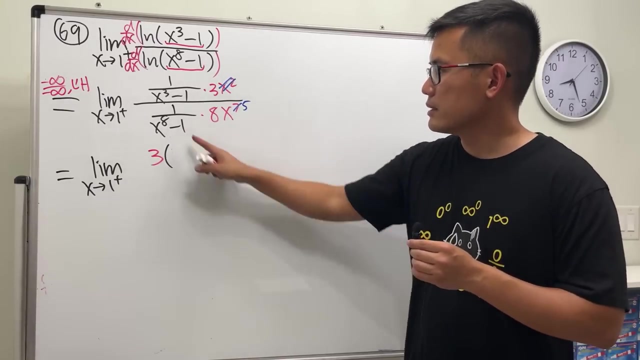 so this is out. right, this is out. this is also x to the five. okay, so i have a three on the top. yeah, i have a three on the top, and then i'm going to bring this up, so it's three times x to the eight minus one, because this right here goes to the top. so it's x to the eight minus one over. 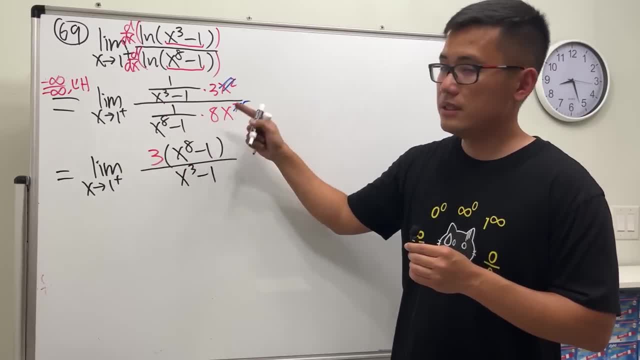 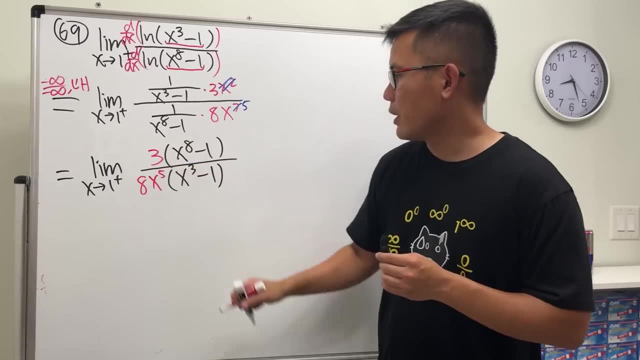 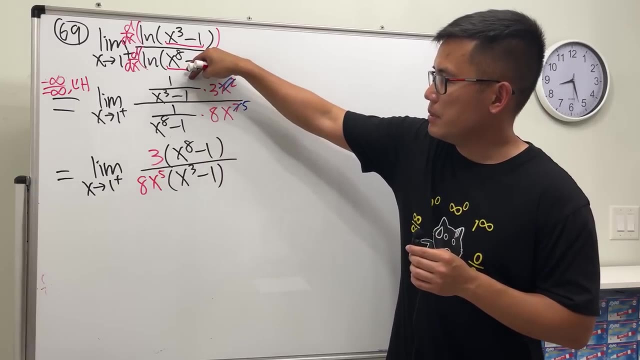 this is on the bottom right. x to the third power minus one, and this is also on the bottom. so i will multiply this with eight x to the fifth power. okay, so kind of verify this on your own. just multiply this, bring that to the top and then three with that, and then eight x to the fifth is still on. 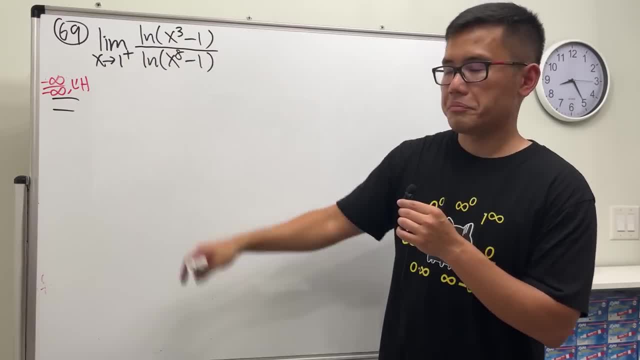 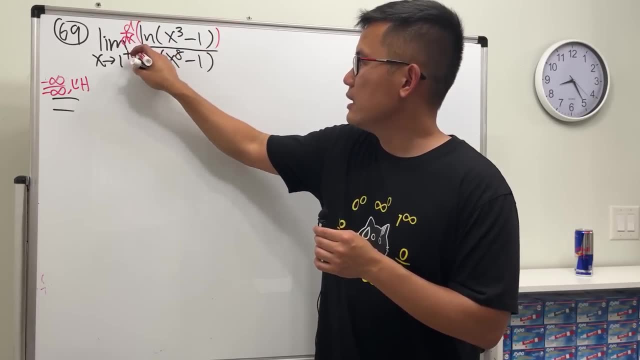 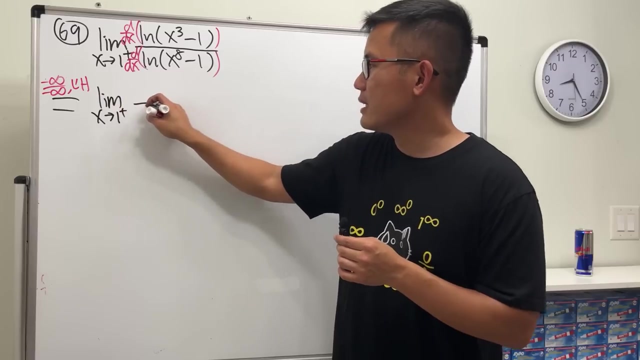 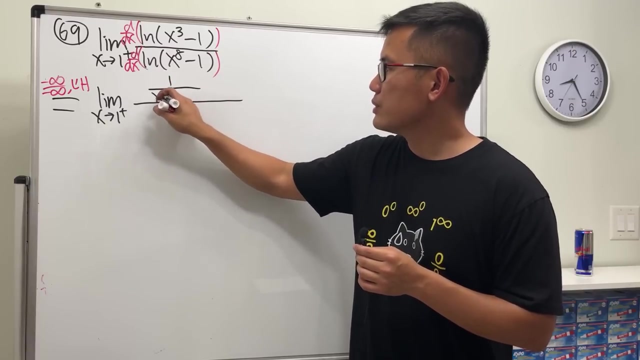 because we get Ln of zero plus. oh, not zero plus. that's why, Anyway, dx, ddx. okay, here we go. Limit x approaching one plus When we differentiate Ln. we just put that on the bottom, so it's one over x to the third power minus one. 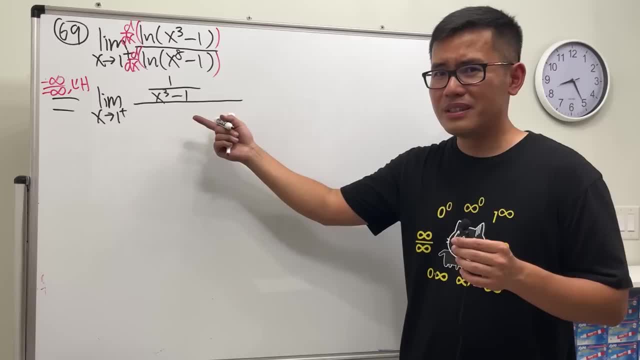 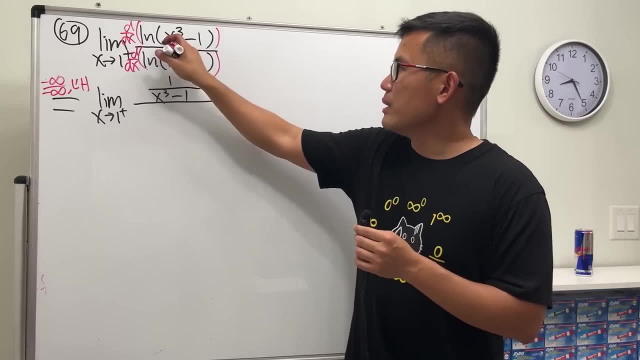 You don't have to multiply by Ln of the base. Technically you do. Ln is log base e. When you have Ln, e is just one, so it doesn't really matter. Anyway, multiply by the inside derivative. That's the chain rule. 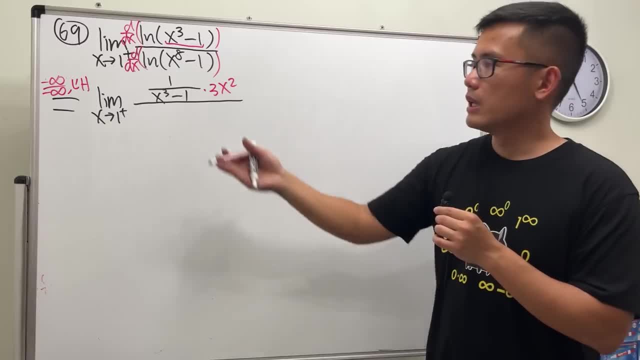 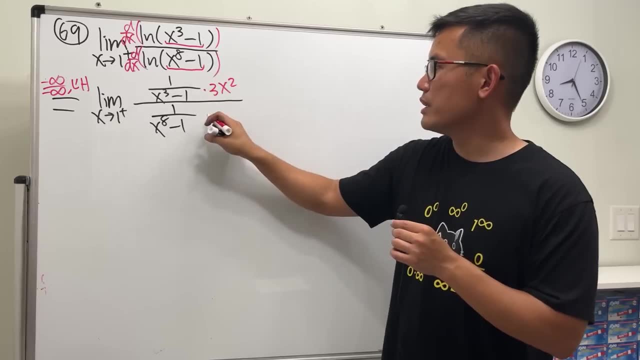 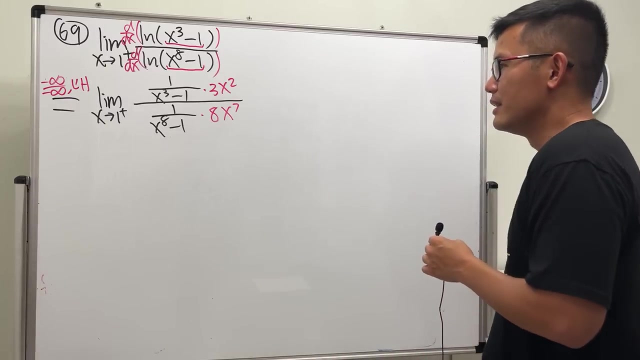 So multiply by three x squared. Do the same thing on the bottom. We get one over x to the eighth power, minus one. and then multiply the derivative on the bottom, which is eight x to the seventh power. Wow, Okay. so what I will do next is: 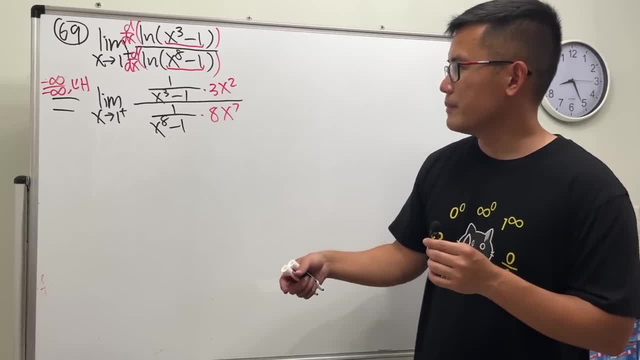 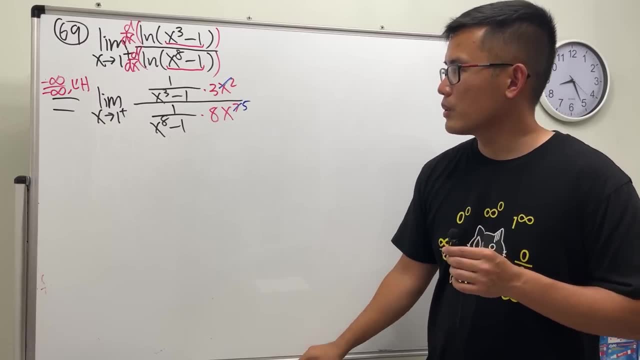 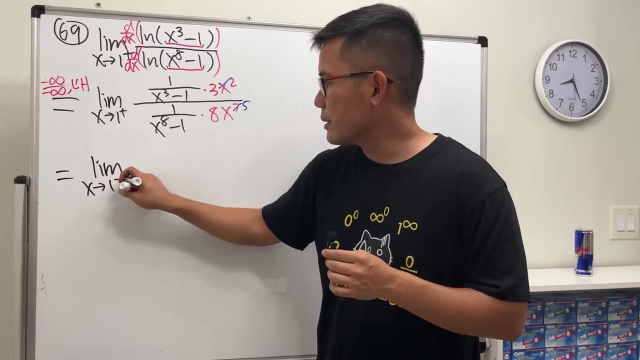 I'm just going to kind of: well, let's reduce this a little bit. yeah, This, and that will cancel. It will become the fifth power, only Cool. And then we are going to get the limit as x approaching one plus. 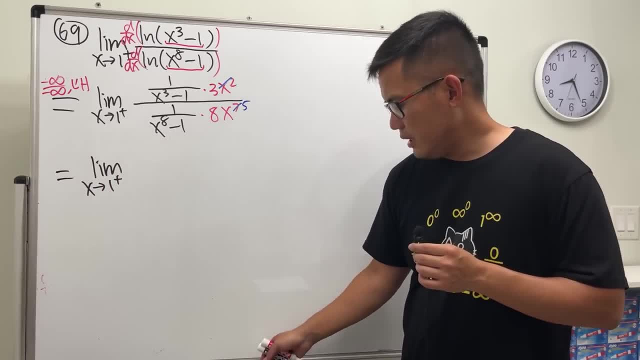 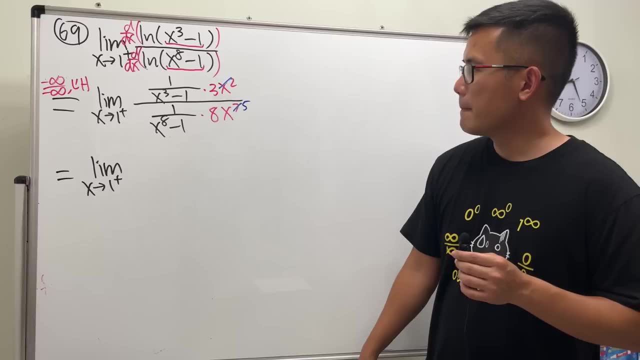 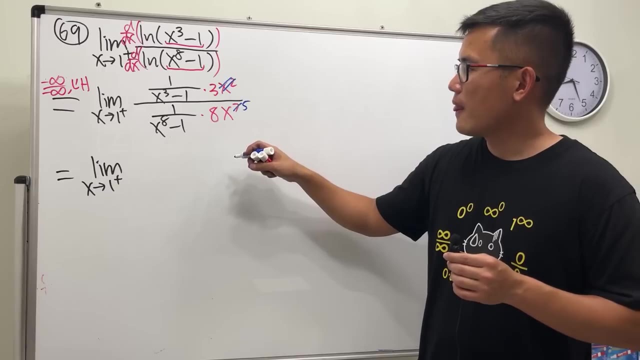 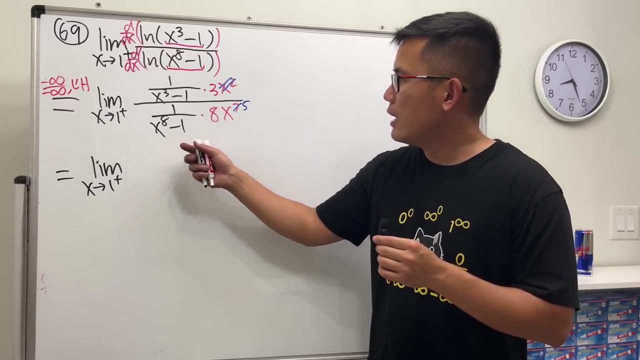 And to make things more clear, I think I'm just going to do the stucy. So this is out. right, This is out. This is also x to the fifth. Okay, So I have a three on the top, yeah. 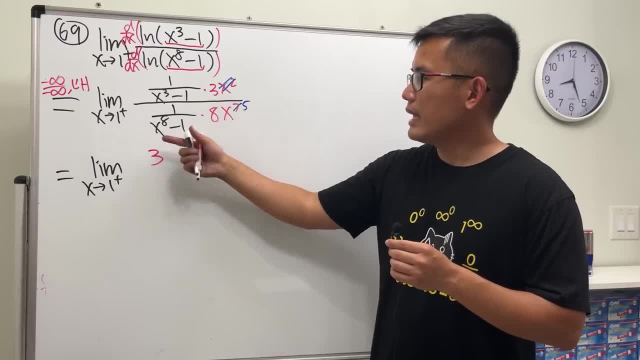 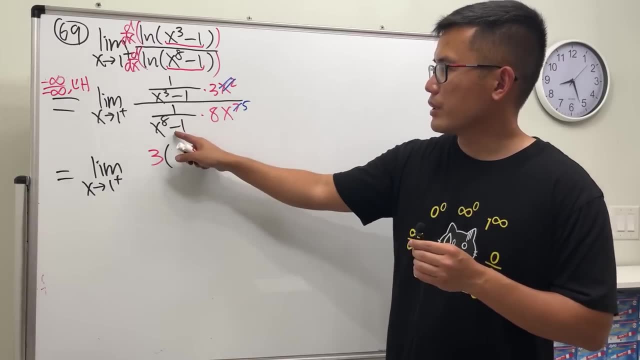 I have a three on the top And then I'm going to bring this up. so it's three times x to the eighth minus one, because this right here goes to the top. so it's x to the eighth minus one over. this is on the bottom right. 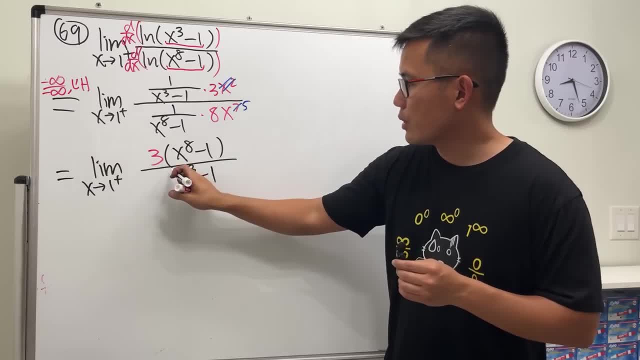 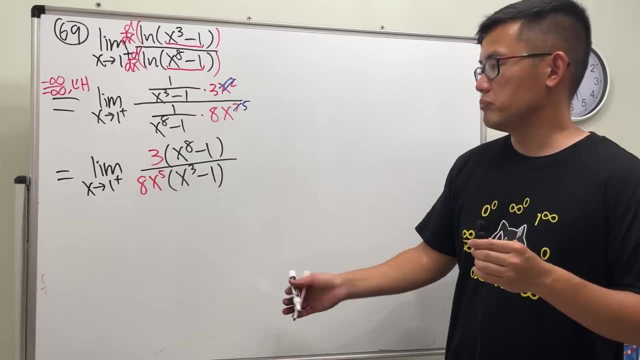 x to the third power minus one, and this is also on the bottom. so I will multiply this with eight x to the fifth power. Okay, So kind of verify this on your own. just to multiply This. bring that to the top. 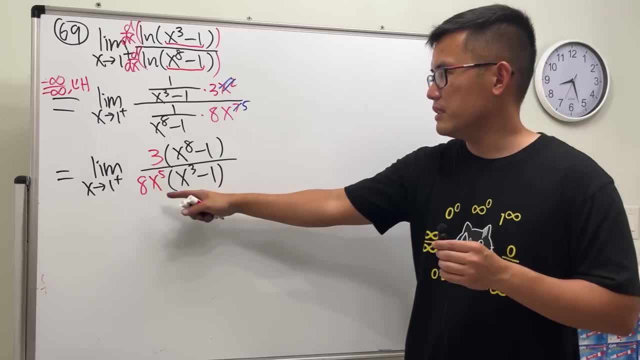 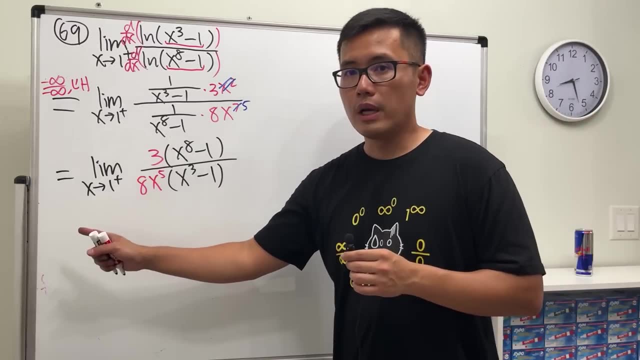 And then three with that, And then eight x to the fifth is still on the bottom along with that, for the denominator Cool x is approaching one. So what we can do next is just multiply out, And then you can do L'Hopital's rule again. 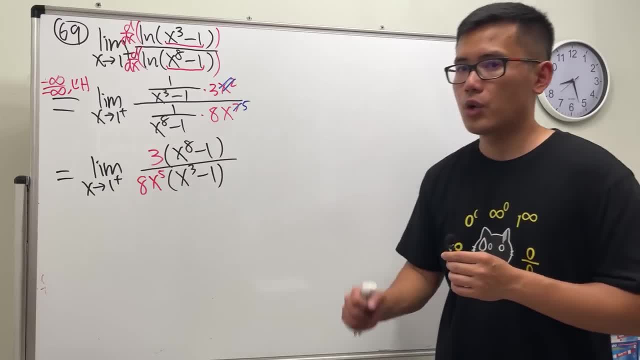 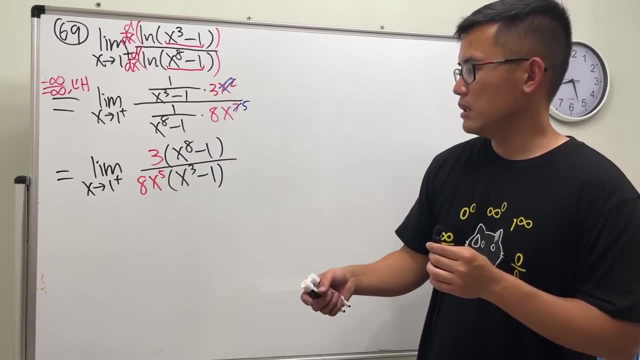 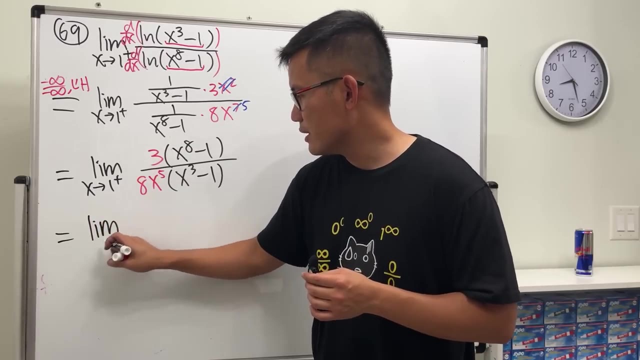 the bottom, along with that for the denominator cool, x is approaching one. so what we can do next is just multiply out, and then you can do lobby toss through again, let's just lapido through again, because why not? but let's multiply this out first. this is the limit as x approaching one, plus we get. 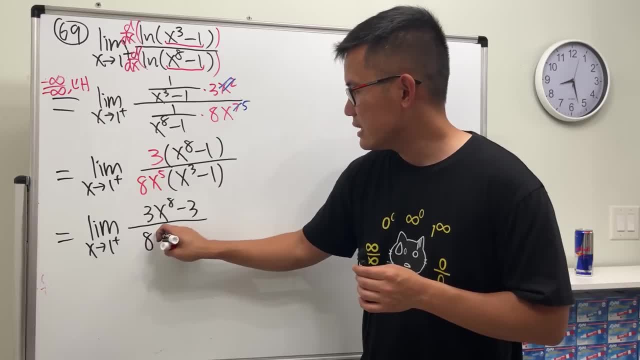 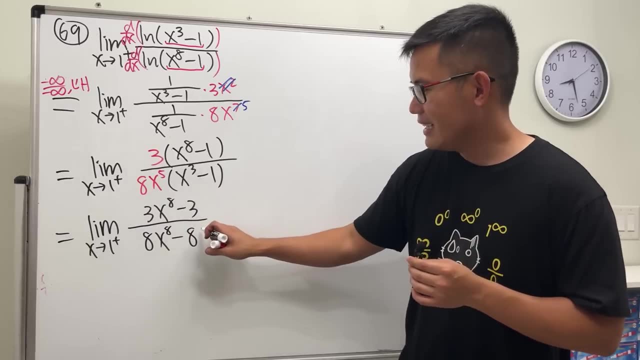 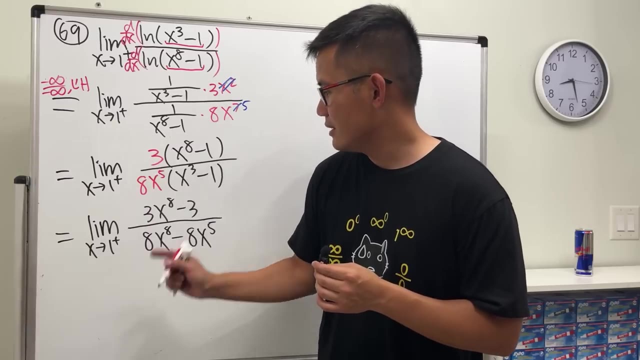 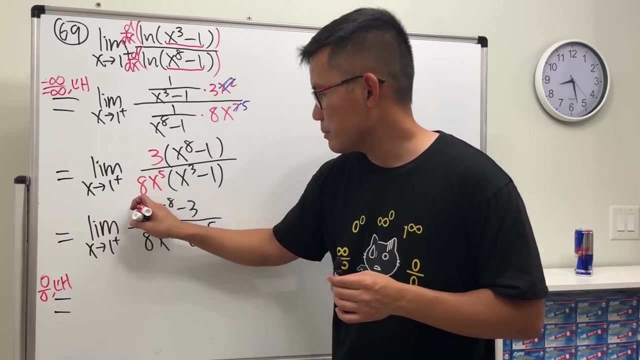 to the eight minus three, and then eight x to the. you add the exponent which is eight minus five minus eight x to the fifth, okay, and then this time we get zero over zero. yeah, so so lapito's rule here, right? well, dtx here, right, dtx. here. we're using lapito's rule for all this. 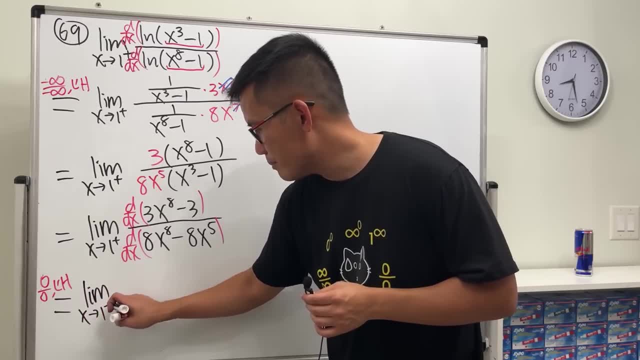 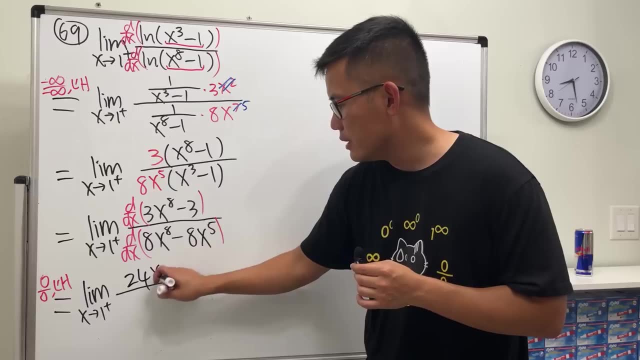 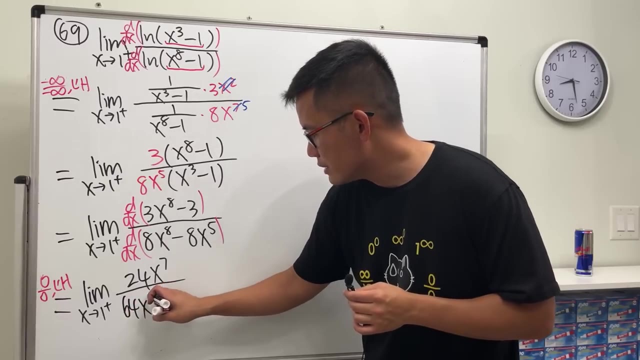 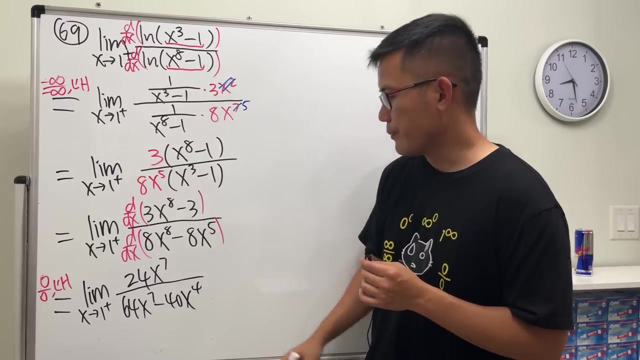 so limit as x approaching one plus the derivative of the half, 24, x to the seven, yeah, zero. bring the a to the front is 64, x to the minus. bring the 5 to the front is 40 and x to the 4.. cool, now we're just going to be plugging. 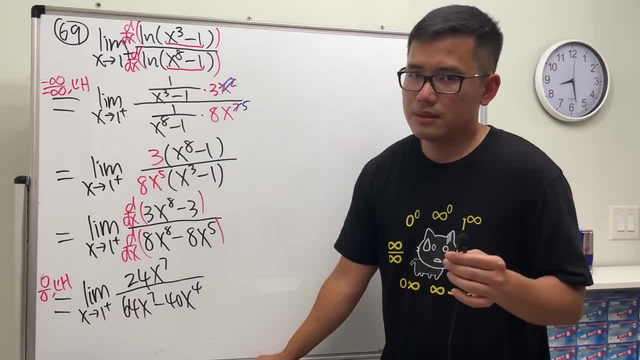 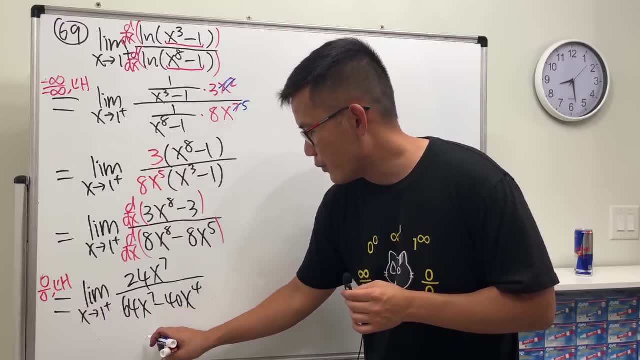 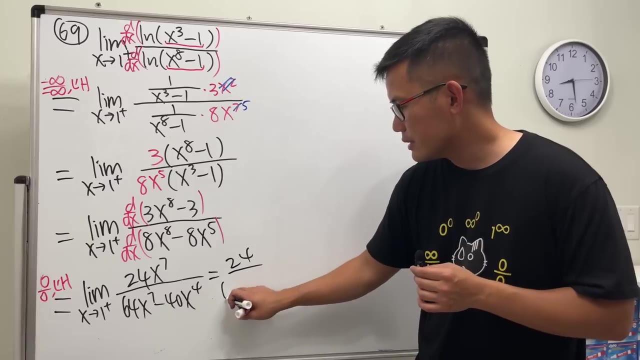 1 into all the x, and then you don't have to reduce or whatnot, because it doesn't really matter that much. but if you look at the bottom, when x is equal to 1 on the bottom, here is just equal to 24, right, yeah, so it's like this: you get 24 over 64 minus 40, so all in all we get 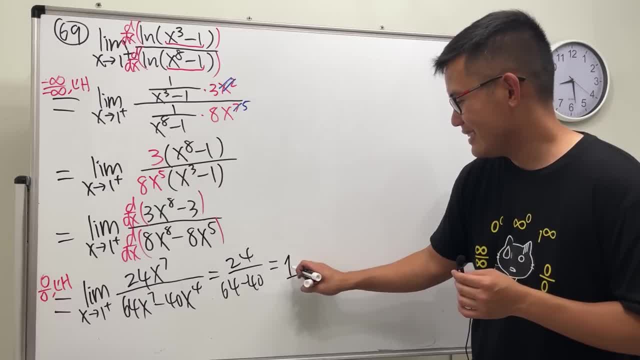 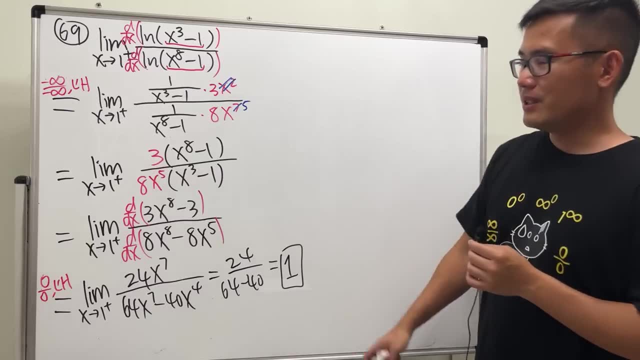 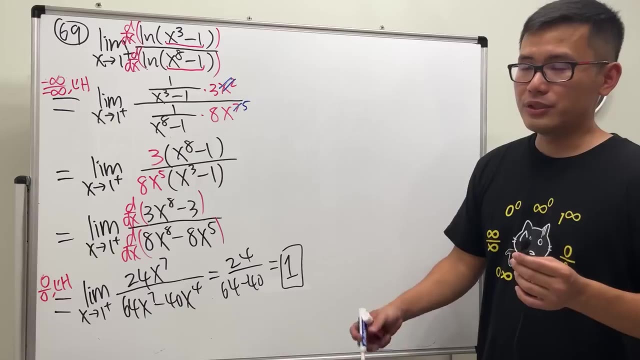 24 for 24.. why am i doing this to myself? that the answer is just equal to 1.. yeah, the answer to this right here is equal to 1.. okay, i have a question for you guys, just to make sure that you guys are actually, uh, paying attention, so go ahead and leave a question, right. 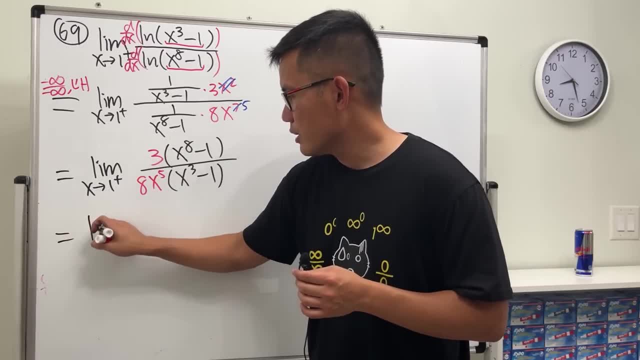 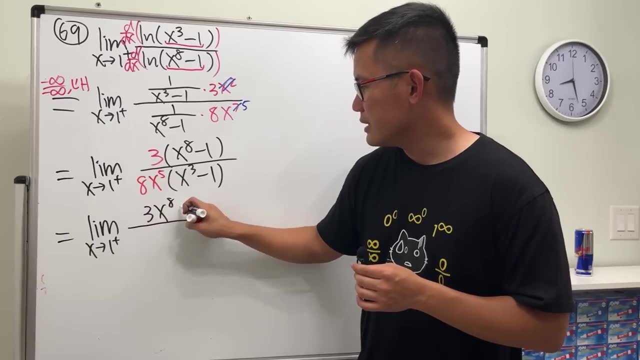 Let's just do L'Hopital's rule again, because why not? But let's multiply this out. first, This is the limit, as x approaching one plus, We get three x to the eighth minus three, And then eight x to the. you add the exponent, which is eight. 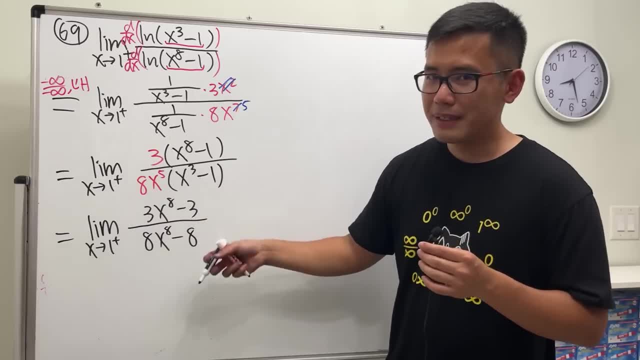 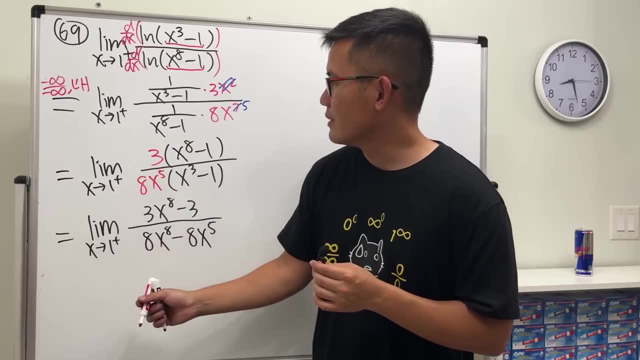 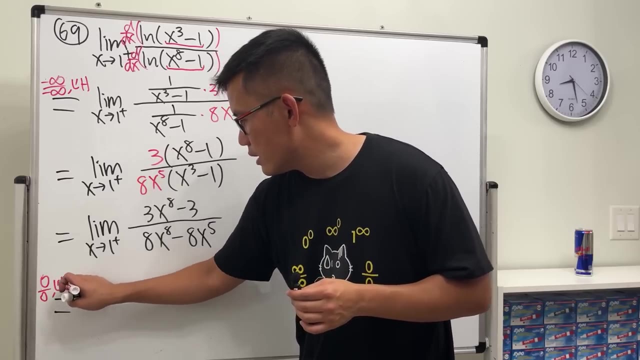 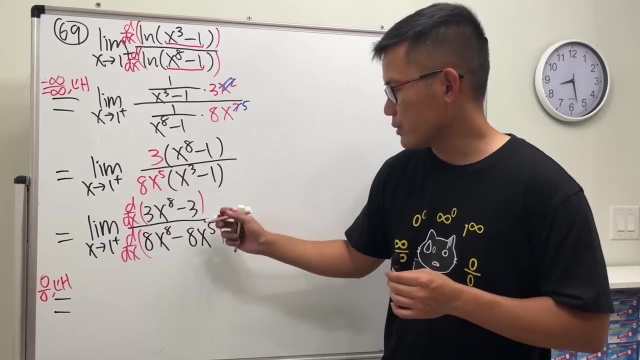 minus five minus eight, x to the fifth, okay, And then this time we get zero over zero, Yeah, So L'Hopital's rule here, right? Well, d dx here, right, d dx. here We're using L'Hopital's rule for all of this. 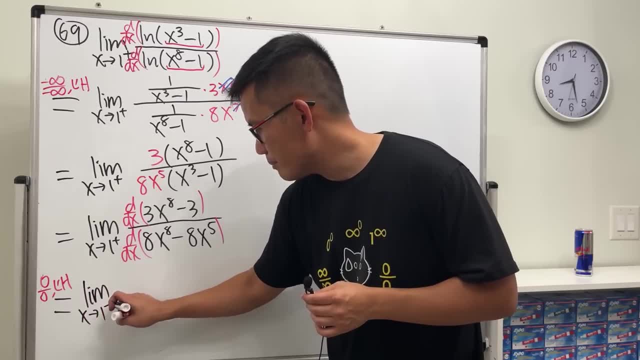 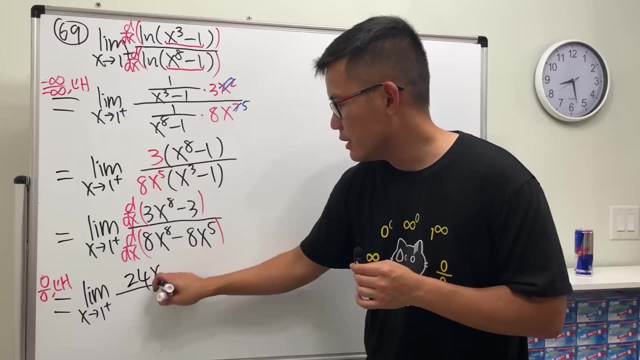 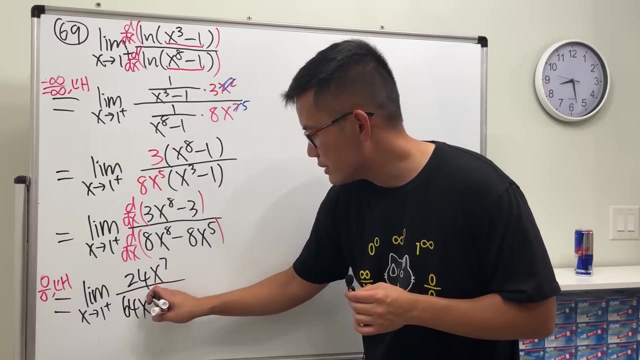 So limit As x approaching one plus the derivative of the half, 24,. x to the seventh, yeah, Zero. Bring the eight to the front is 64,. x to the seventh minus Bring the five to the front is 40, and x to the fourth. 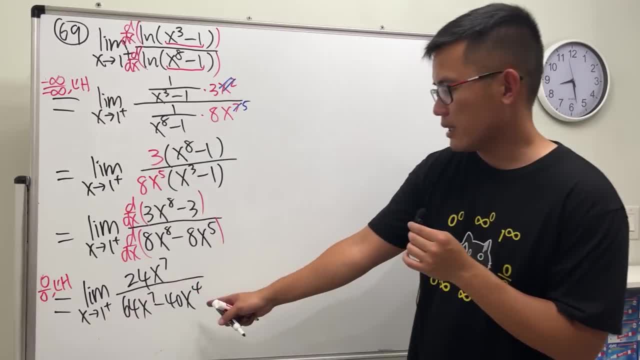 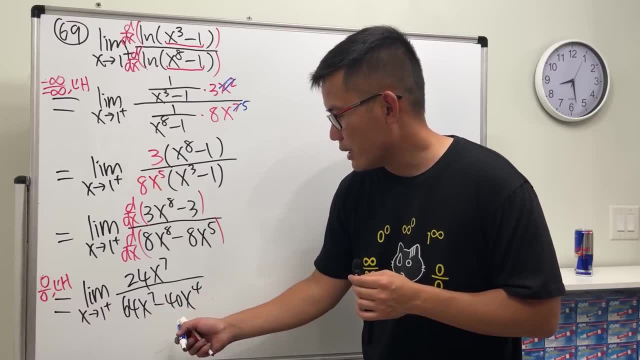 Cool, Now we're just going to be plugging one into all the x And then you don't have to reduce or whatnot, because it doesn't really matter that much. But if you look at the bottom, when x is equal to one, 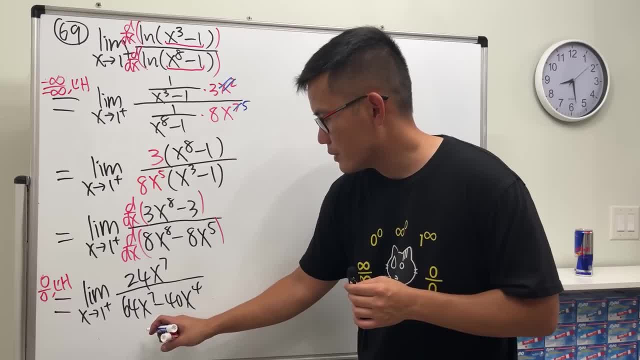 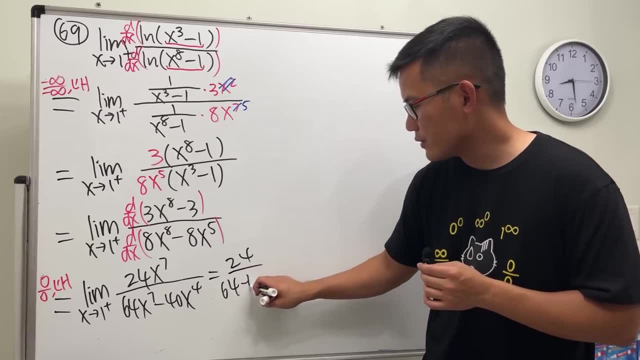 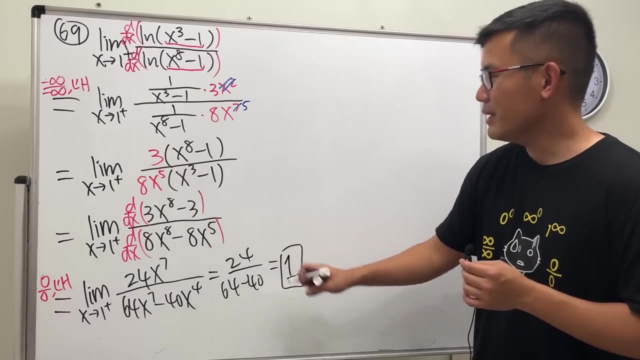 on the bottom here, it's just equal to 24, right, Yeah? So it's like this: You get 24 over 64 minus 40. So all in all, we get 24 over 24.. Why am I doing this to myself that the answer is just equal to one. 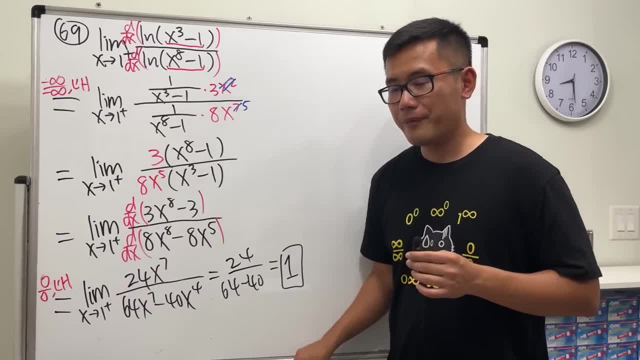 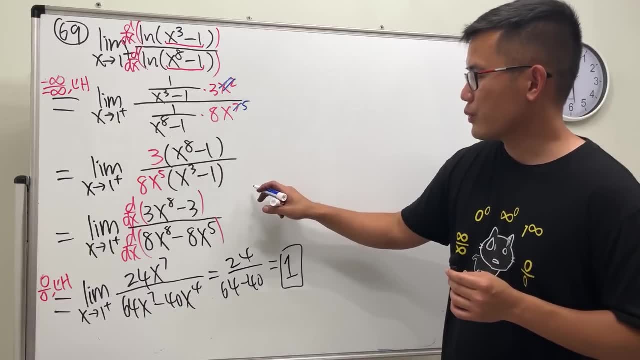 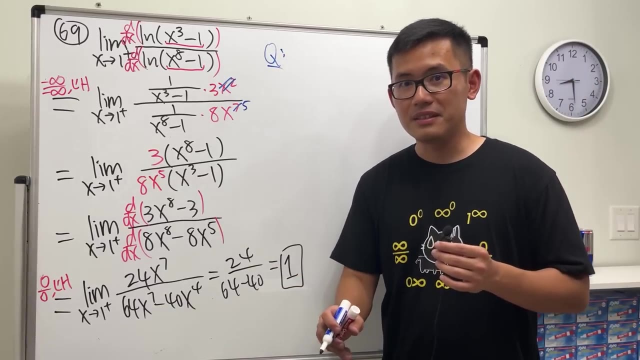 Yeah, The answer to this right here is equal to one. Okay, I have a question for you guys, just to make sure that you guys are actually paying attention. So go ahead and leave a question right here. right, Leave the time stamp and then leave the answer. 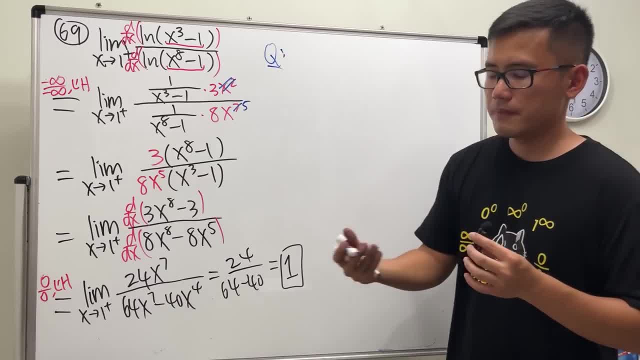 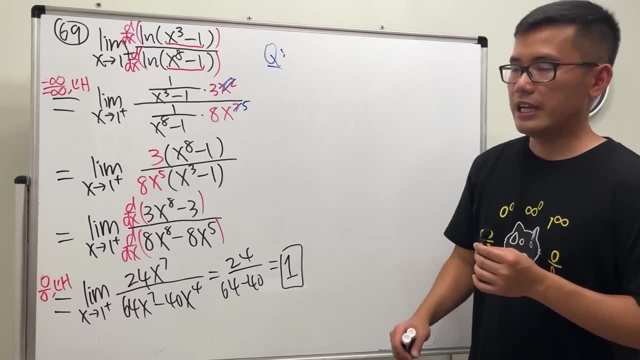 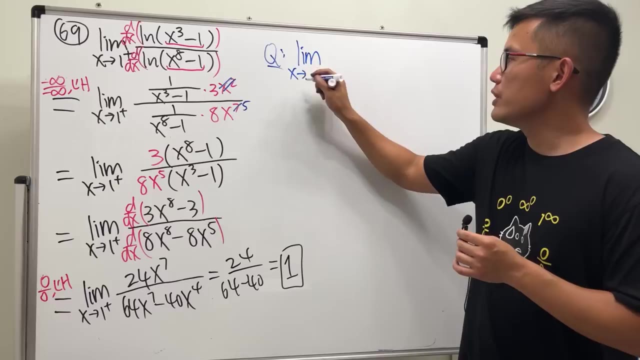 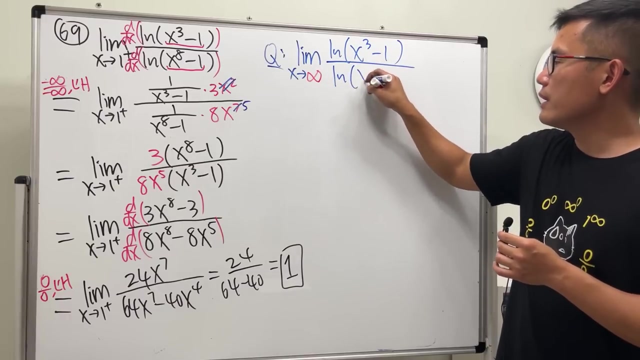 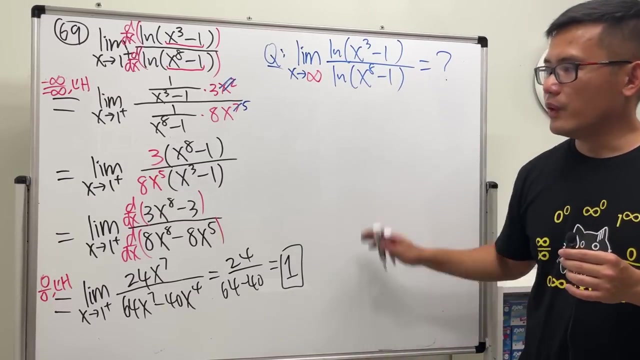 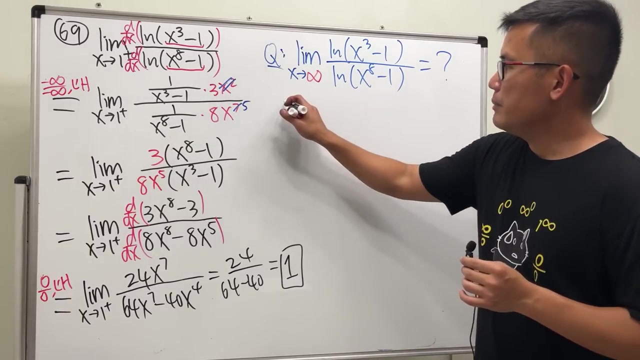 here right now, leave the timestamp and then leave the answer. i want you guys to try this. we just take your rage, find it 8, 5 in 5, 6, 4, 15, 16, 16, 27, 28, 28, 32, 33. 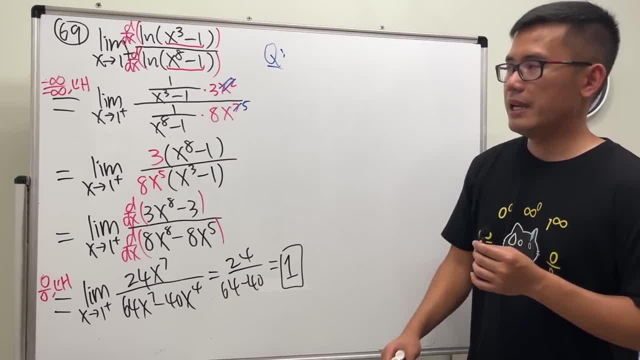 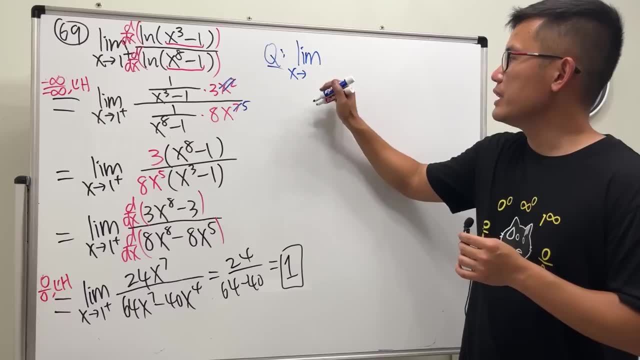 I want you guys to try this. I want to keep the function the same, but instead of x approaching one plus, go ahead and figure out what if we have the limit as x approaching infinity And then we have ln of x, x to the third power minus one. 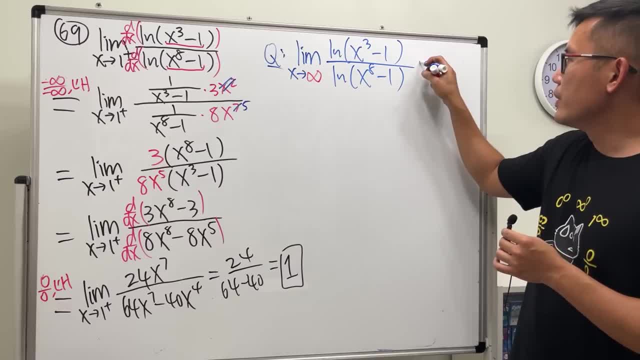 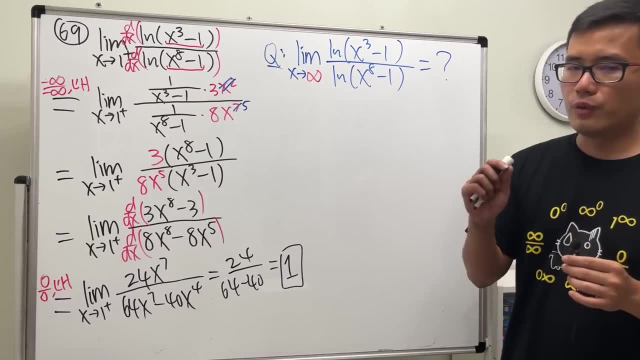 ln of x to the eighth power minus one. Okay, You guys do it. The work is almost identical, but you have to be really careful of one little place, and then you should be able to figure this out. I am going to squeeze in number 70 here. 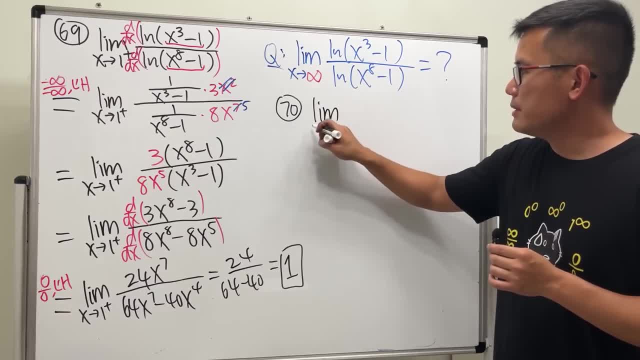 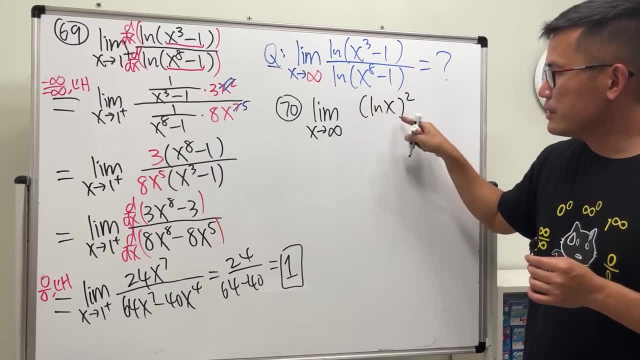 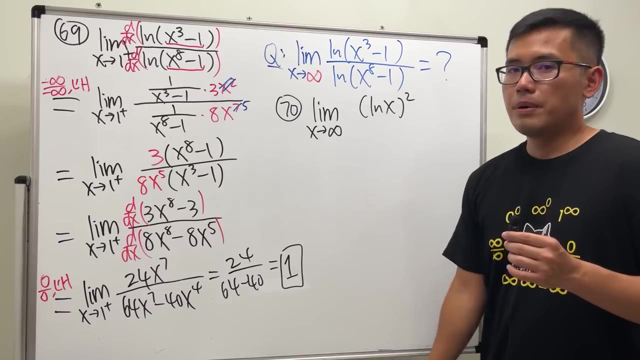 because I want to, I really want to Limit x approaching infinity. We have ln x, This is ln xn squared, So I am going to use the power rule here, So do not bring the two to the front as like the log. power rule. 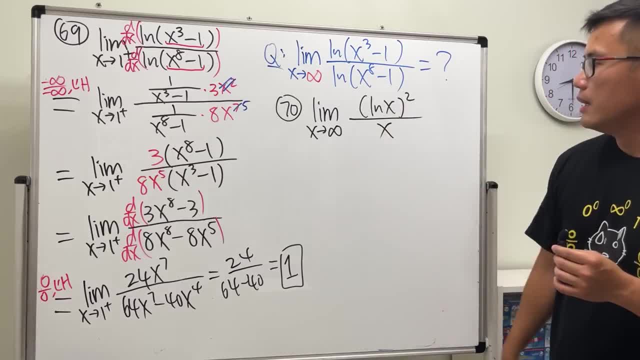 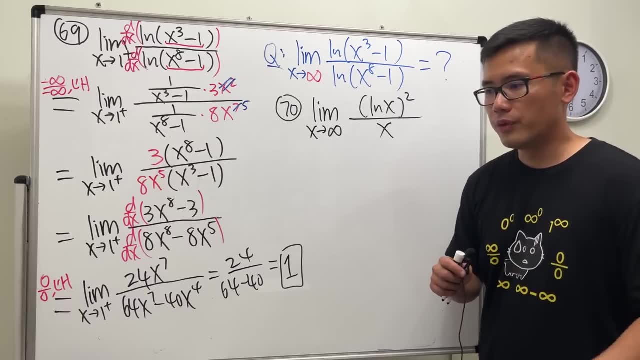 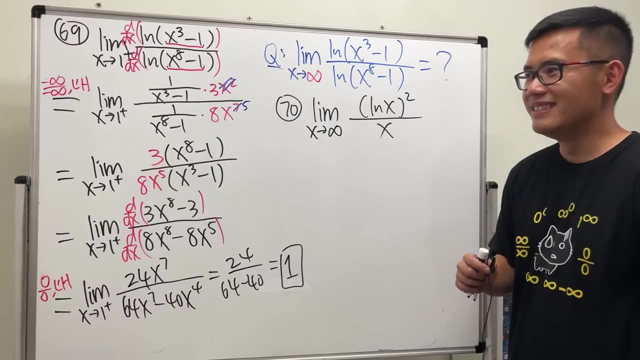 Don't do that. alright, This is x, But anyway, though, we will use the power rule for the derivative, but not the power rule for the logarithm. So pay attention to the following: How late, Anyway? infinity into here. 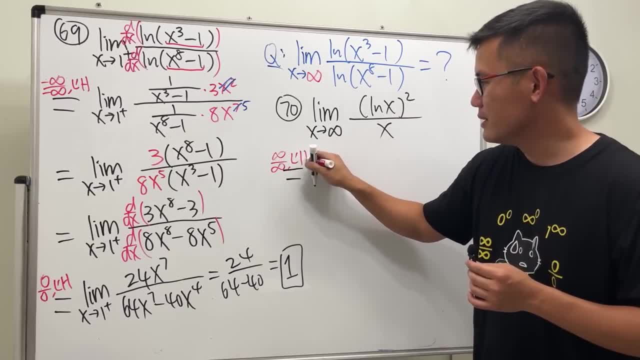 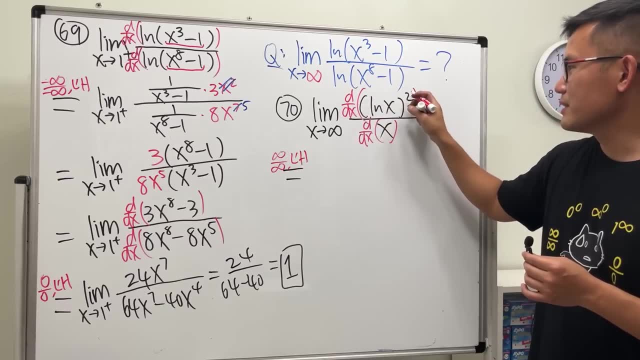 you get infinity over infinity. So Lapito's rule, Last question of Lapito's rule, man Yay, Because it just has a lot of things to write. Anyway, bring this to the front at minus one. Here we are looking at. 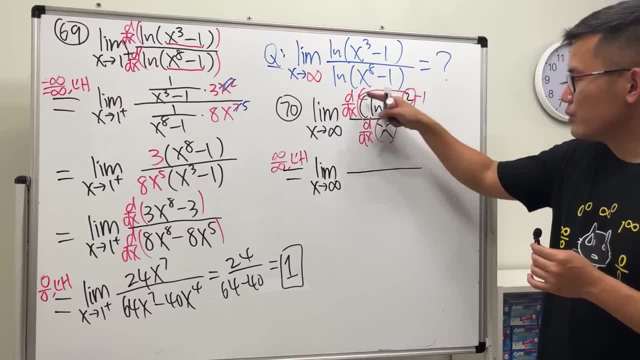 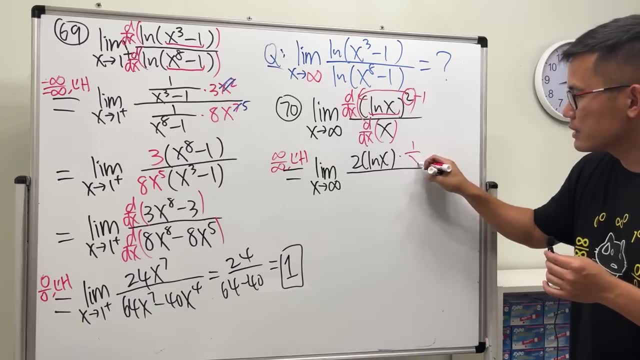 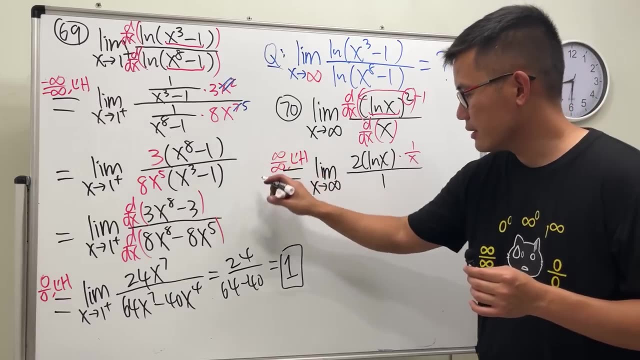 limit as x approaching infinity two to the front, ln, x, and then multiply the derivative inside, which is one over x. The derivative of x is just one. So the truth is this right here requires Lapito's rule again. 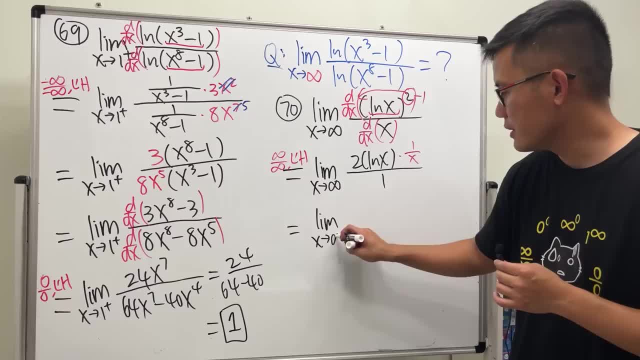 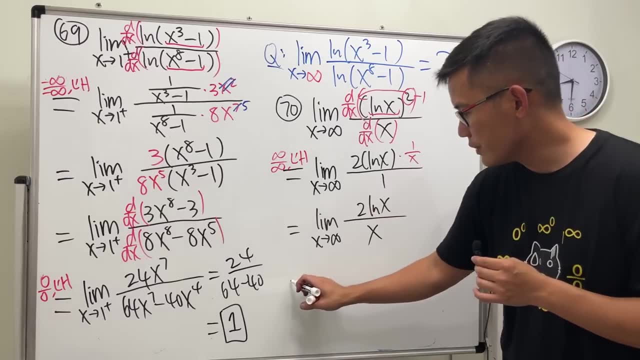 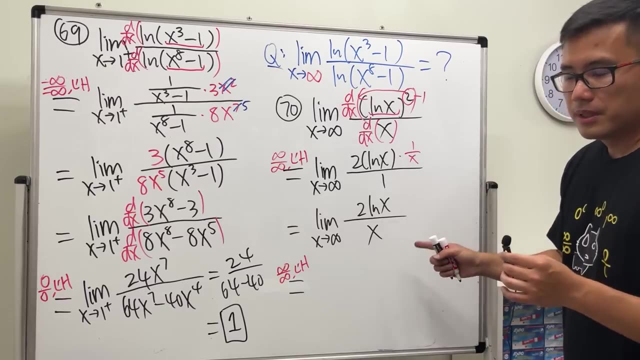 So this right here is the limit as x approaching infinity, two x, no two ln x and over x. right Put infinity, we get infinity over infinity. So Lapito's rule again, And please pay attention to this question. 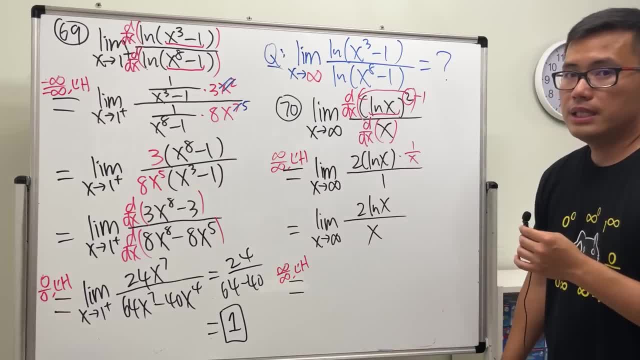 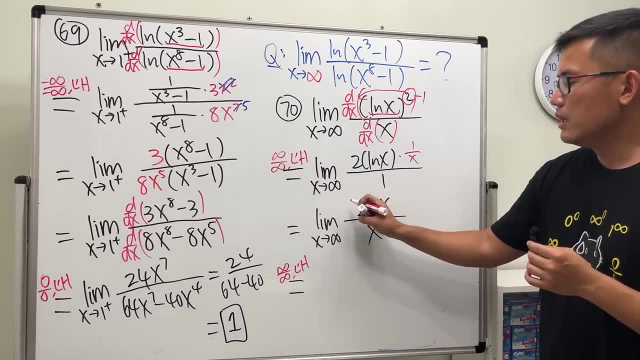 because you will see that we have infinity over infinity, right, This is ln x compared with x. The two doesn't really matter, But let's just do Lapito's rule here: d, dx, d, dx. Here we get a limit. 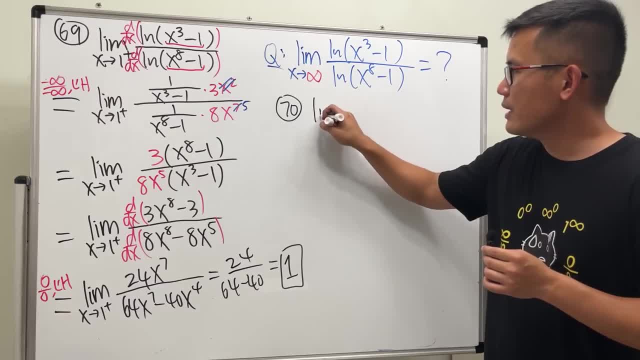 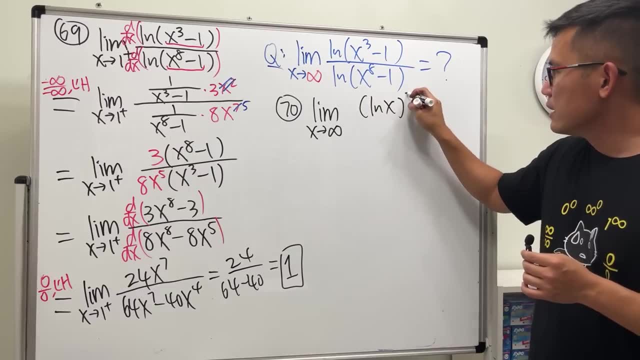 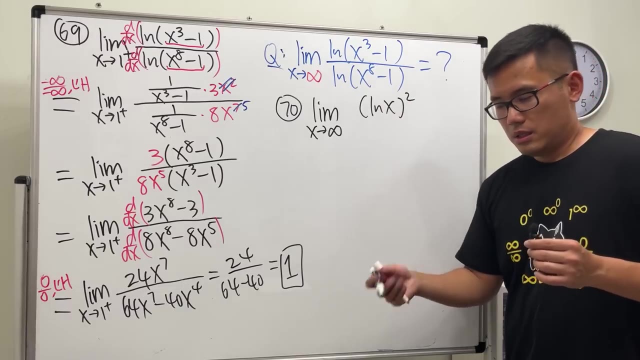 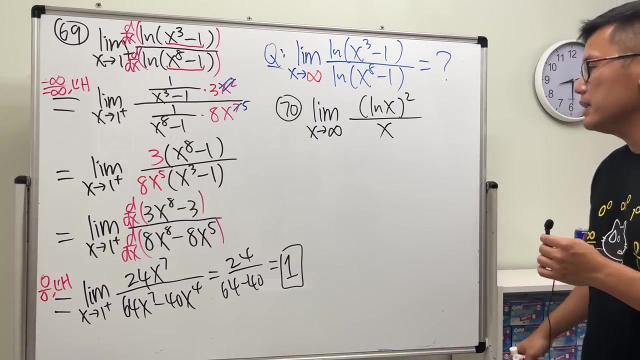 32, 47, 32, 70 here, because I want to, I really want to limit X approaching infinity. we have L and X. this is L and X and the square, so do not bring the two to the front as like the log power rule. don't do that. all right, but anyway, though, we will use. 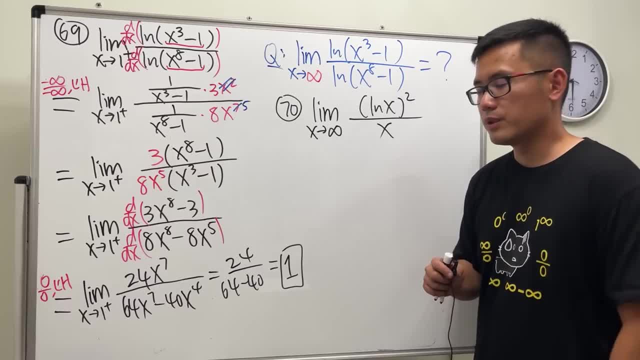 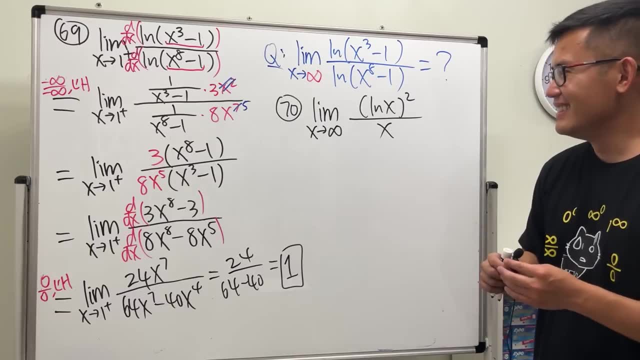 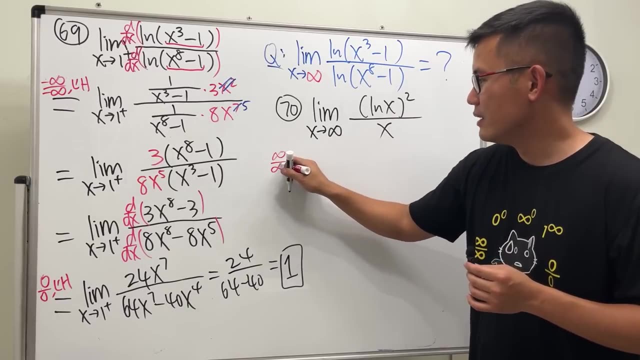 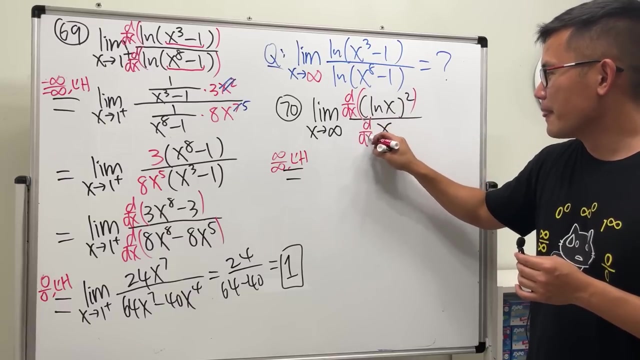 the power rule for the derivative, but not the power rule for the logarithm. so pay attention to the following: holy anyway, infinity into here you can, infinity over infinity. so Lapido's rule. last question of our people's room. and yeah, because it just has a lot of things. 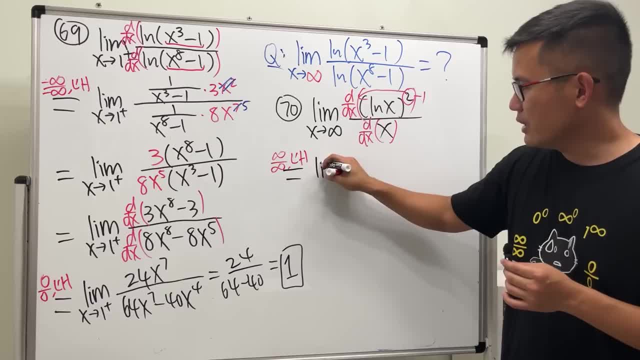 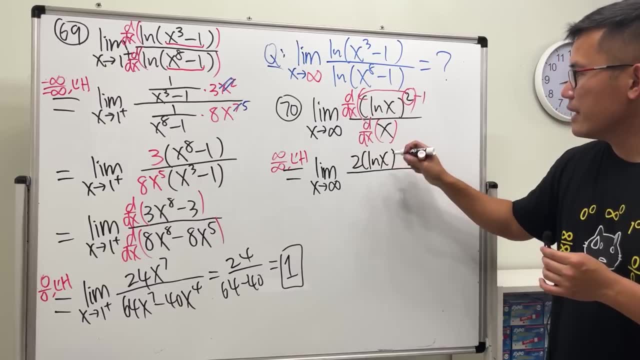 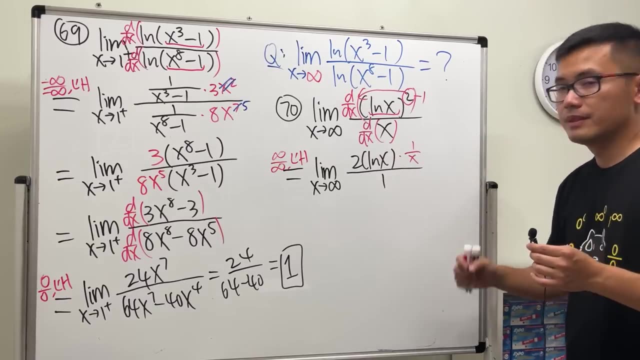 to right. anyway, bring this to the front and minus one. here we are looking at the limit as X approaching infinity. two to the front, L and X, and then multiply the derivative inside, which is one over X. the relative X is just one. but the truth is this right here requires Lapido's rule again. 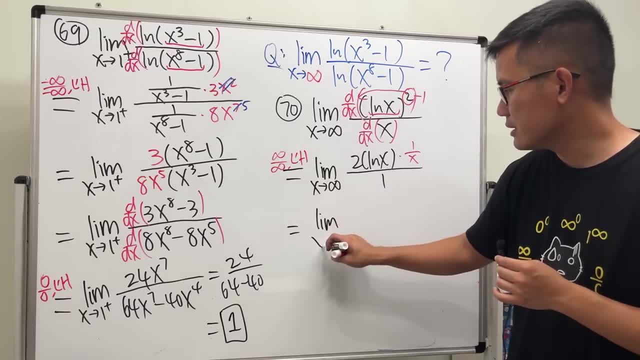 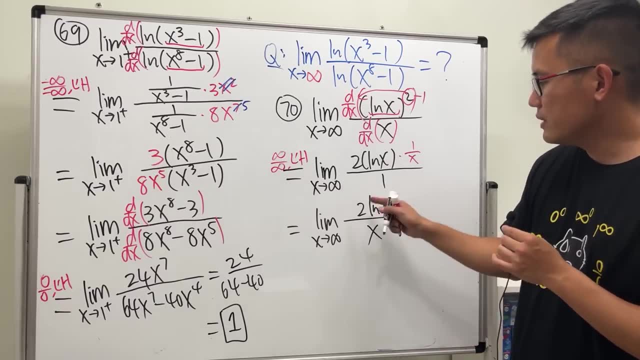 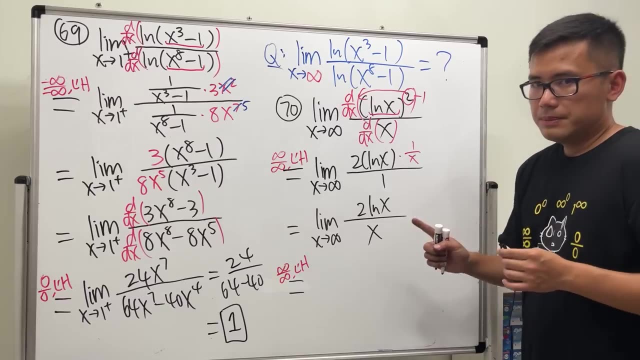 so this right here is the limit as X approaching infinity to X, to L and X and over X, right put infinity. we can't infinity over infinity. so a lot people throw again, and please pay attention to this question because you will see that we have infinity over infinity, right. 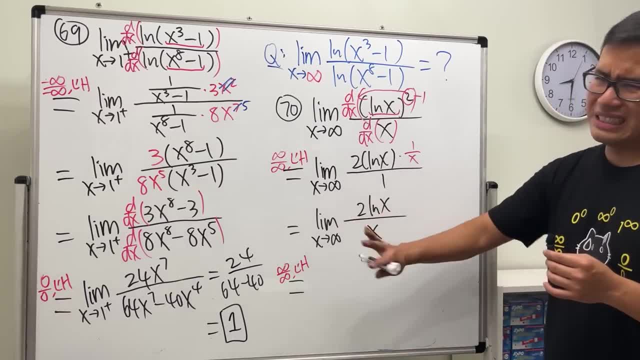 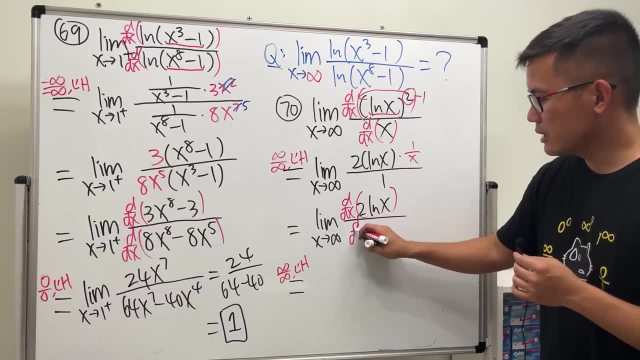 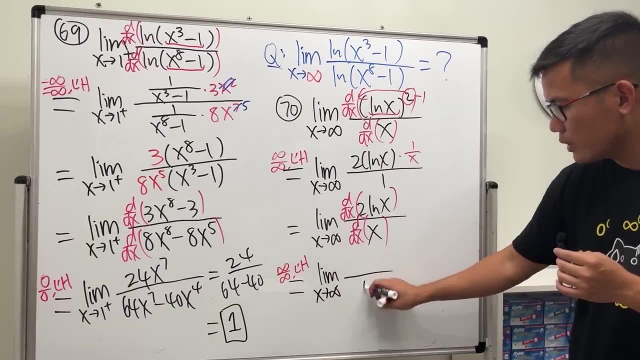 this is our next computer with X. the two doesn't really matter, but let's use to la pito's rule here, D, DX. here we get a limit of stepsuperb, slow P, toastyелиppx wind to the right of the spectrum as X approaching infinity. on the bottom, we get 1. on the top we get 2 times the. 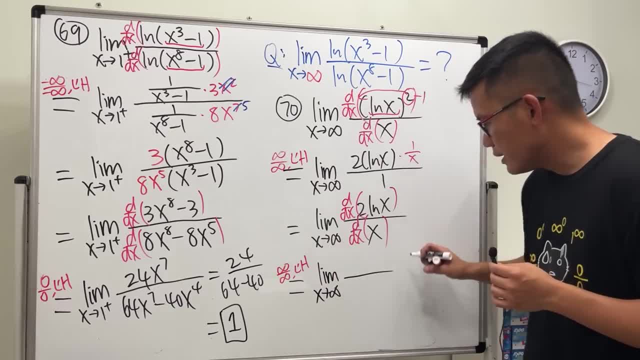 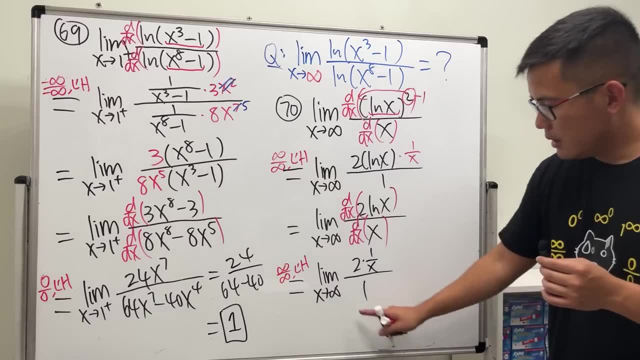 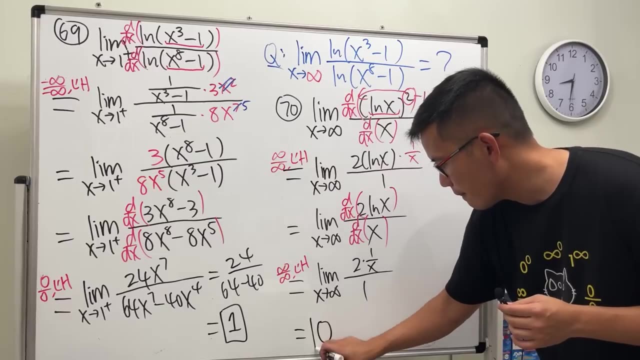 as x approaching infinity. On the bottom, we get one. On the top we get two times the derivative of that, which is one over x. When we put infinity to here, we get two over infinity, Just zero. So what does this mean? 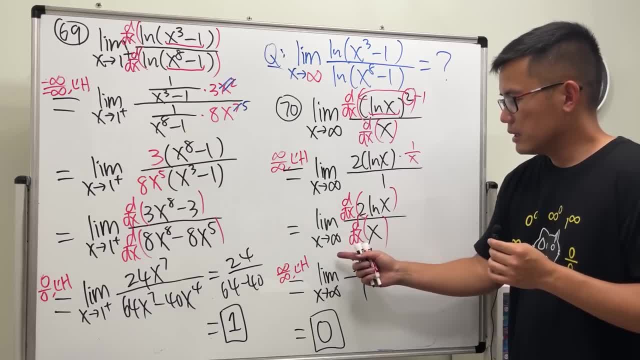 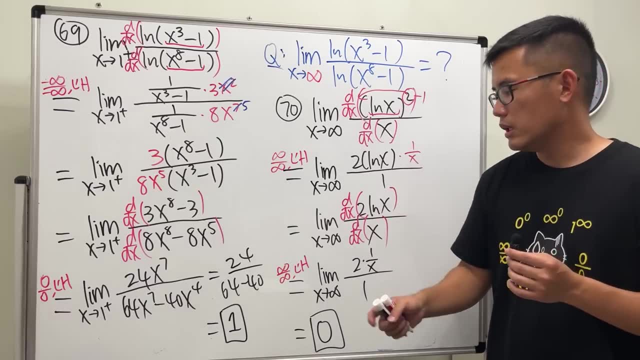 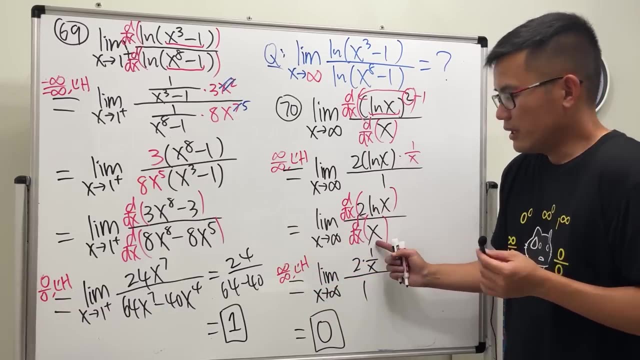 If you look at this, the limit of the ratio of two ln x over x is zero. This means ln x is actually so, so, so small, even though it goes to infinity as well. but this infinity is nothing compared to when x is going to infinity. 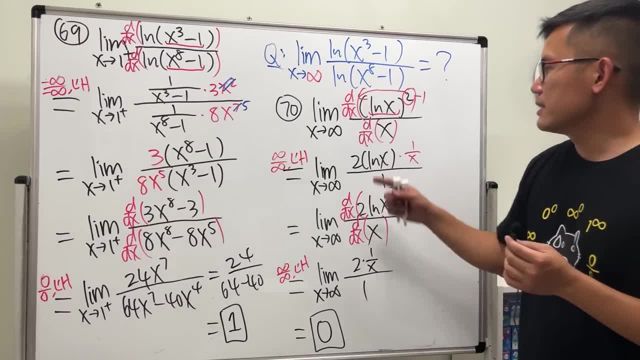 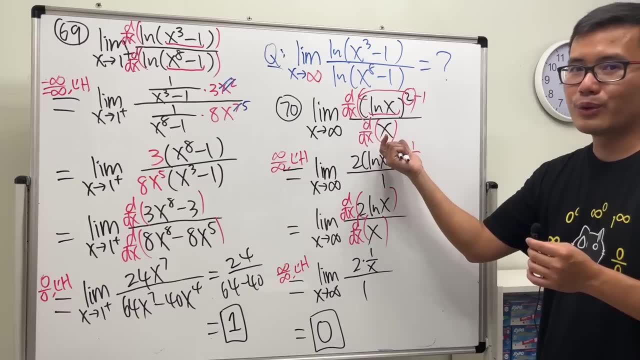 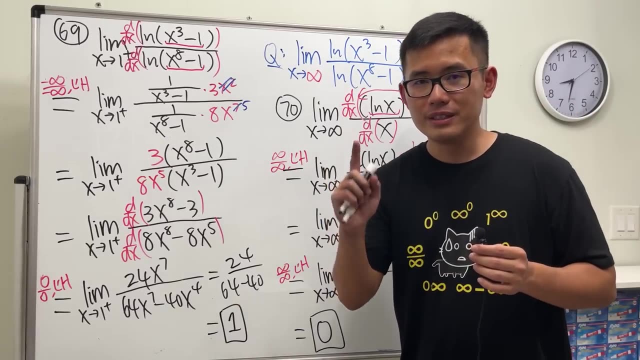 that kind of thing. In fact, you can have ln x to whatever power that you want That will not be bigger than x to some power, Yeah, like a power function. So keep that in mind because, with that being said, we are going to get into the secret weapon. 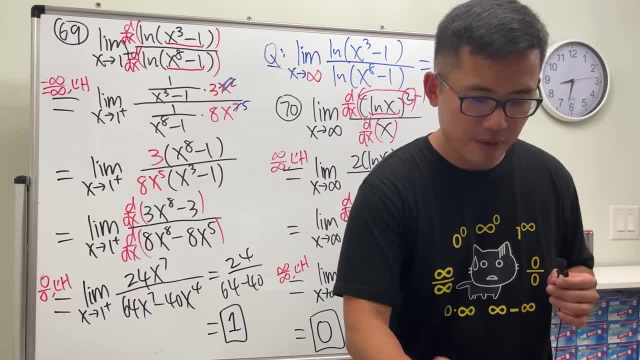 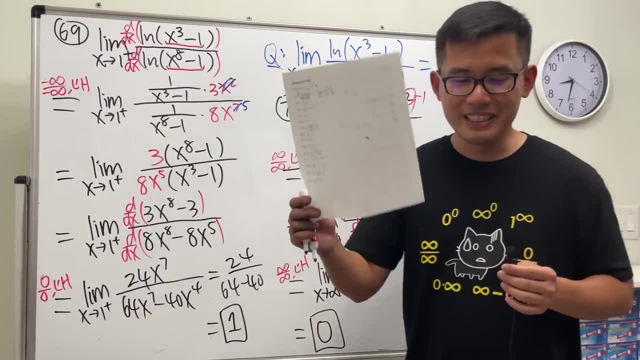 If you know the secret weapon, we will be able to finish a lot of the questions in no time, And congratulations to myself. I finished page six. 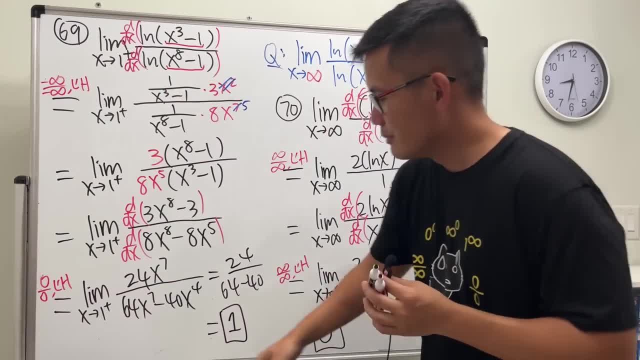 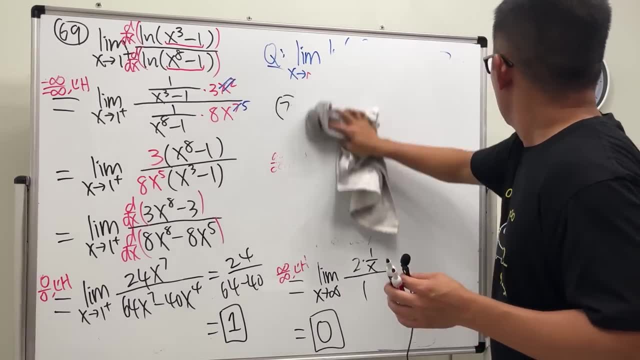 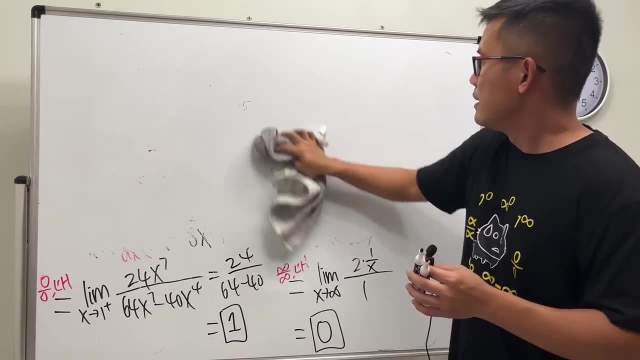 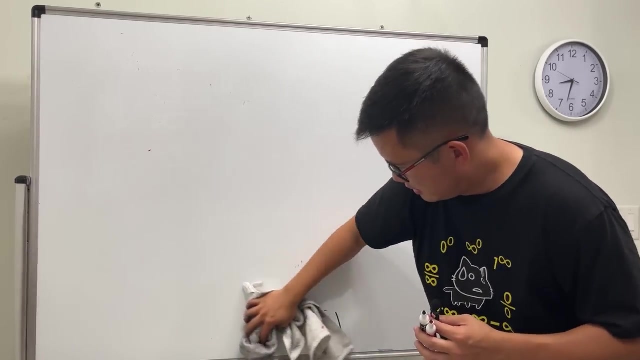 Five hours, Oh, my God. 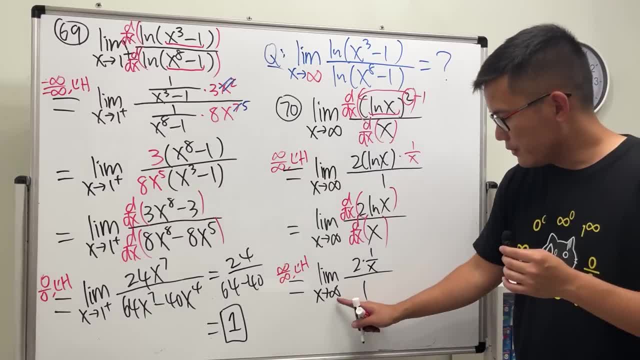 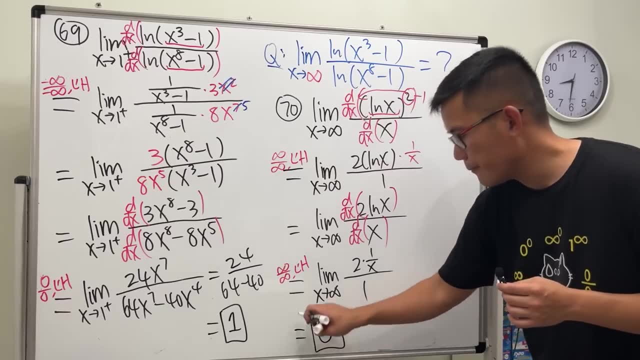 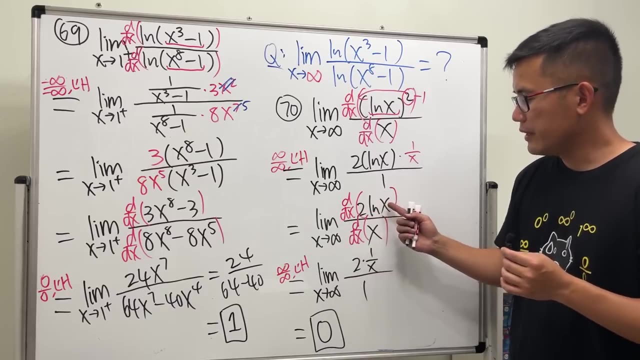 derivative of that which is 1 of X. when we put infinity to here, we get 2 over infinity to 0. so what does this mean? if you look at this, the limit of the ratio of 2 ln X over X is 0. this means ln X is actually so, so, so small, even though 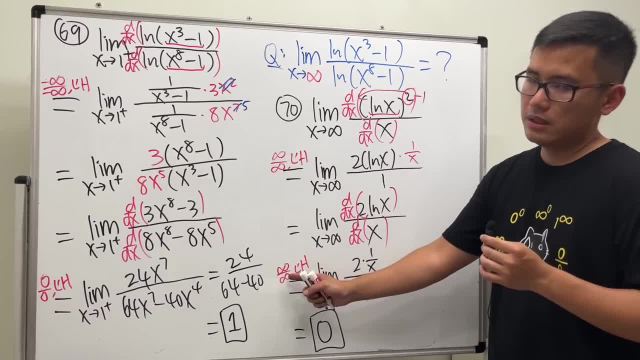 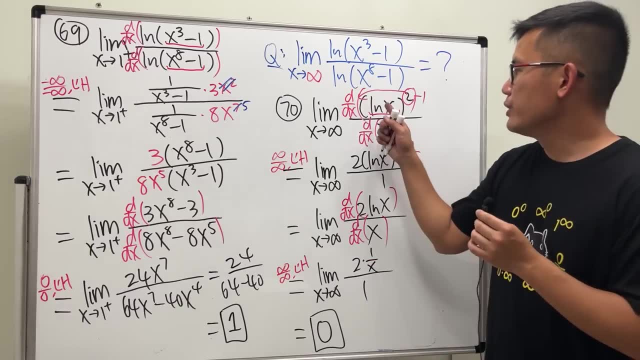 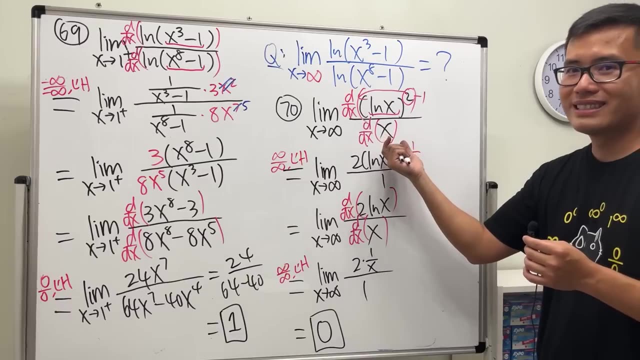 it goes to infinity as well, but this infinity is nothing compared to when X is going to infinity, that kind of thing. in fact, you can have ln X to whatever power that you want. that will not be bigger than X to some power- yeah, like a power function. so keep that in mind because, with that being said, we are 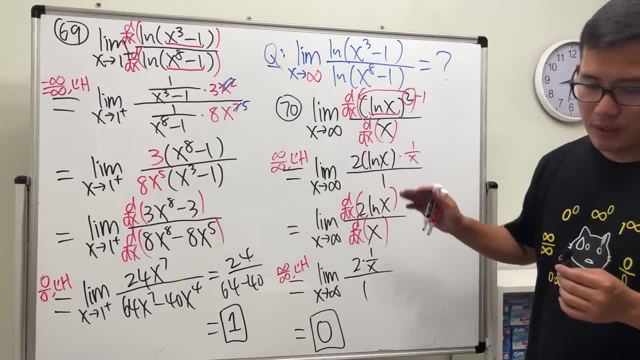 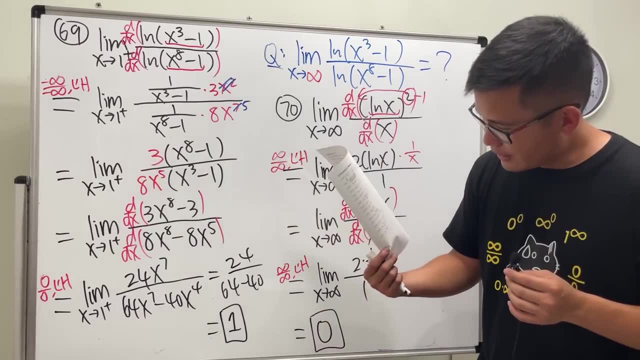 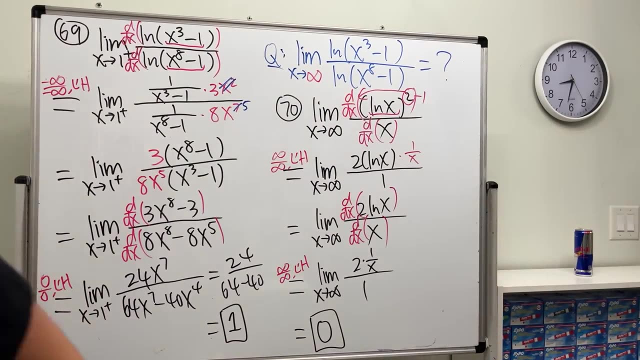 going to get to the end of this video and I will see you in the next video. again to the secret weapon. if you know the secret weapon, we will be able to finish a lot of the questions in no time. and congratulations to myself, I finished page six. five hours, oh my god. 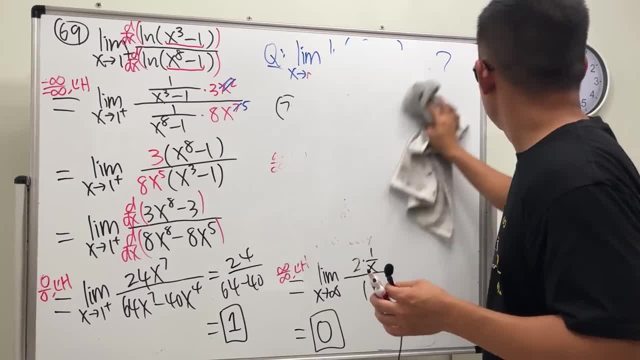 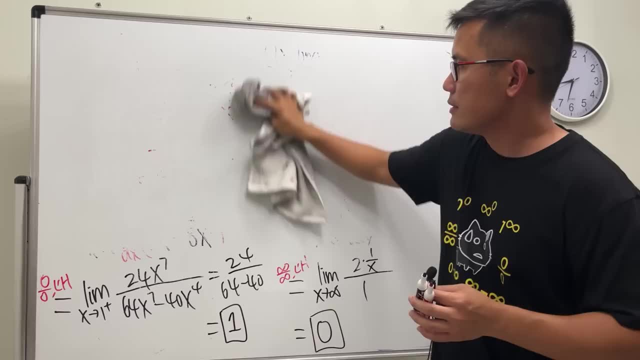 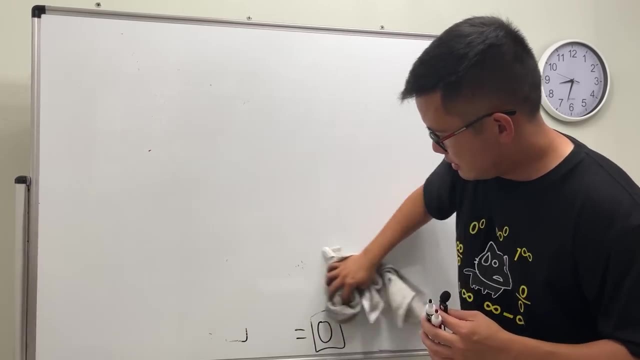 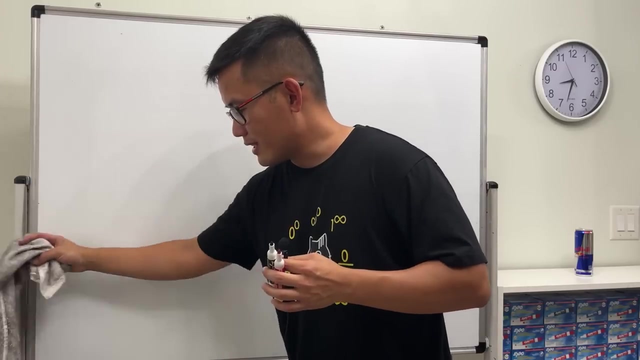 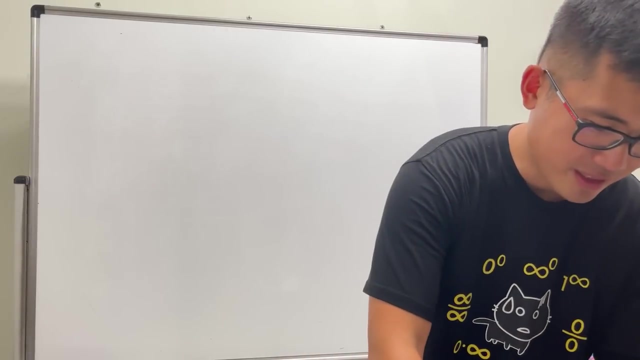 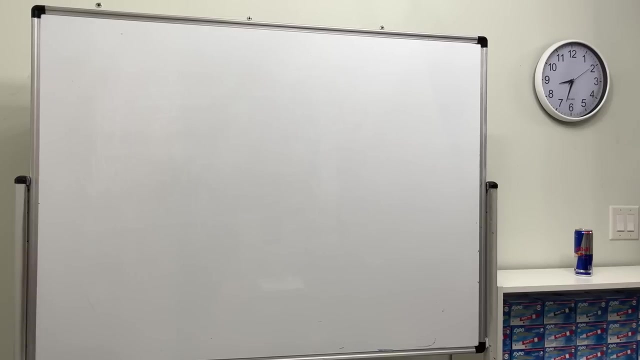 all right, I feel like drinking some soda, so just give me a little bit of a drink and I'll see you in the next video. and I'll see you in the next video. and I'll see you in the next video. I have this, haha, and I'll see you in the next video. 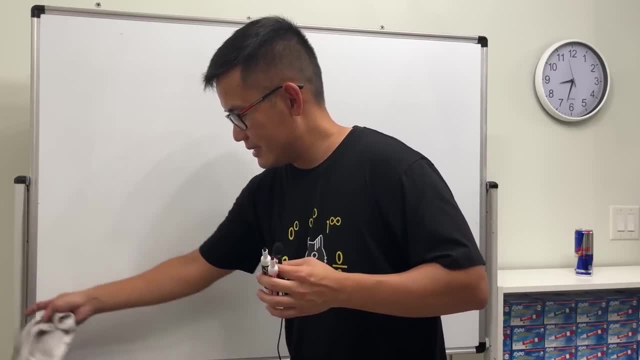 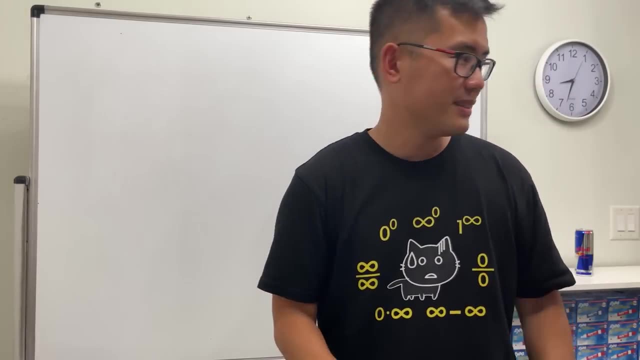 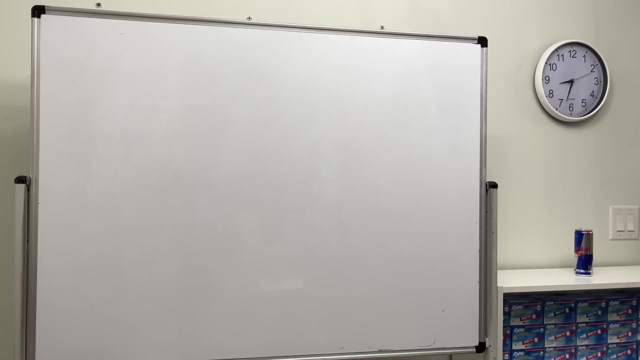 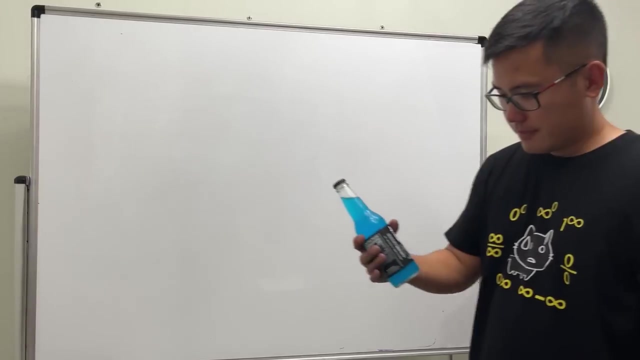 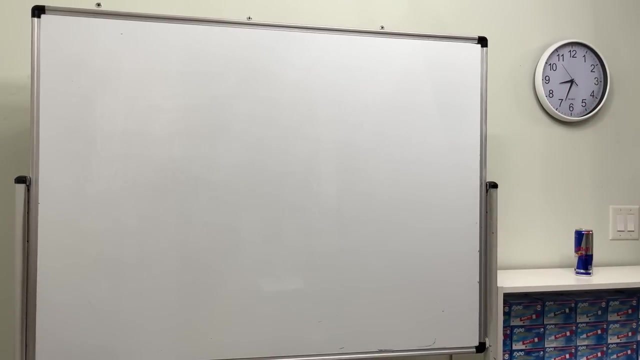 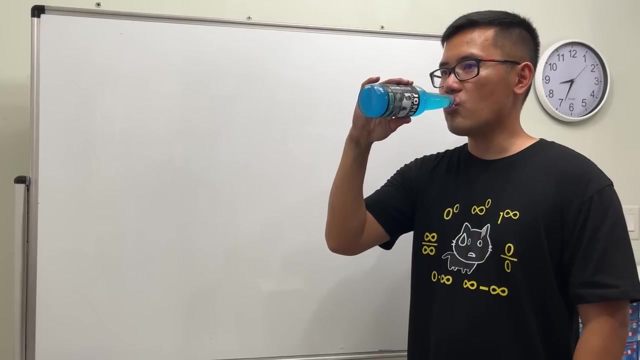 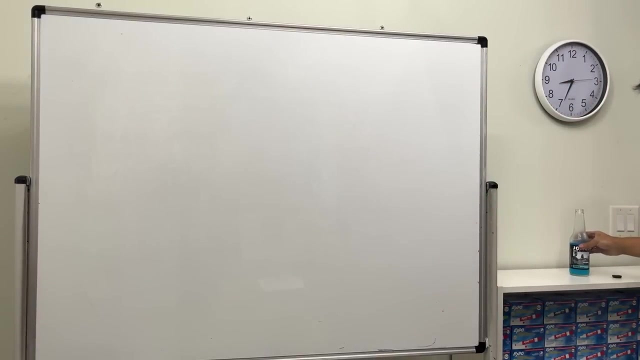 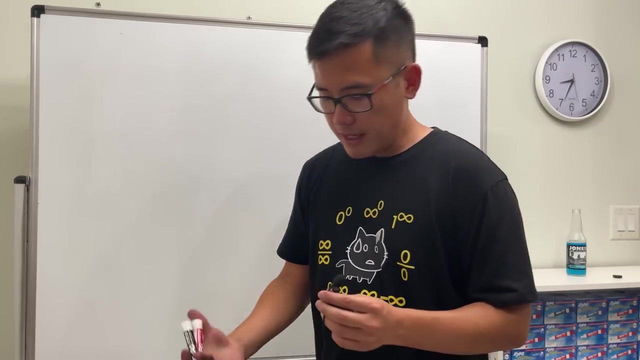 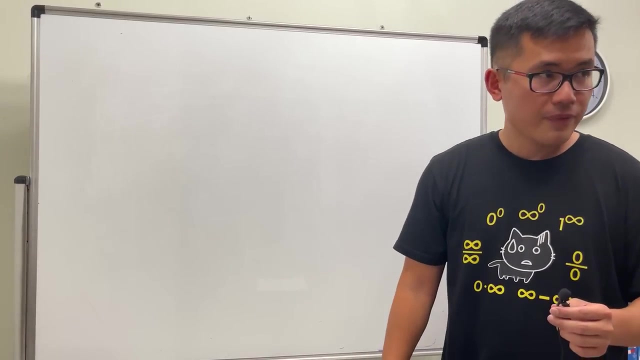 Alright, I feel like I'm drinking some soda, so just give me 20 seconds or so. hmm, i have this, haha. so, oh, he says it's real, but not instead by real. anyway, i should have balsam gatorade. i forgot it's hot. 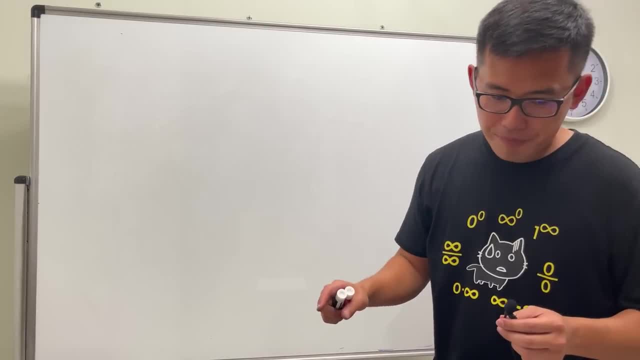 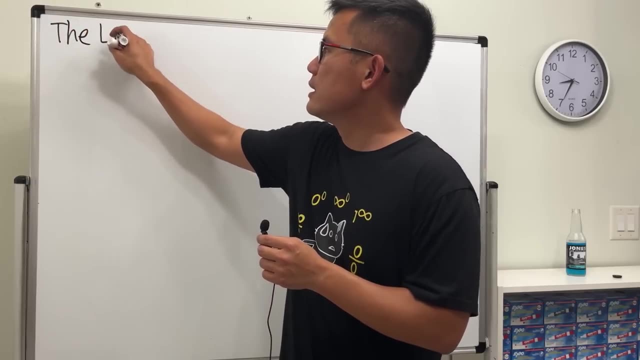 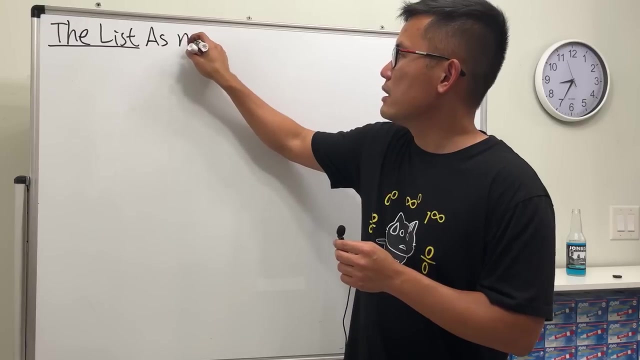 yeah, that's why i have to drink something. but anyway, though, 30 more questions. secret weapon number one: i call this the list. what's the list? well, this is to compare the kind of infinity. i'm using n right here, because this way i can also bring. 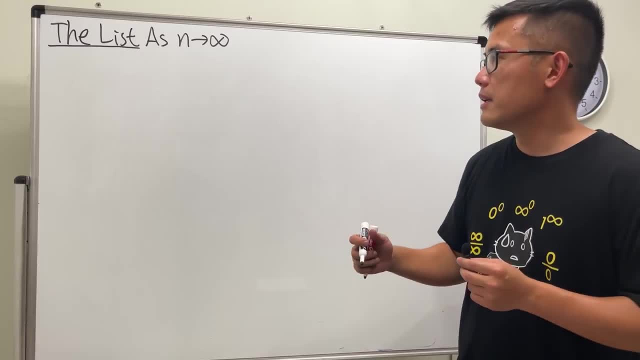 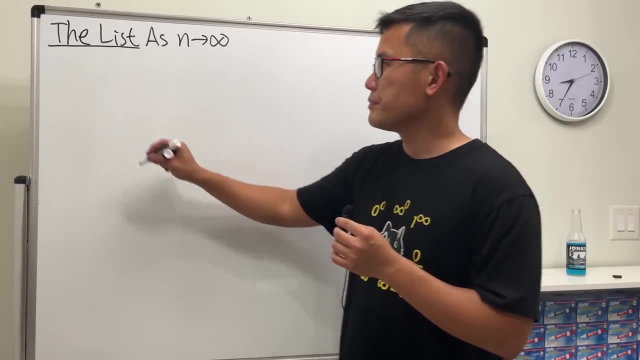 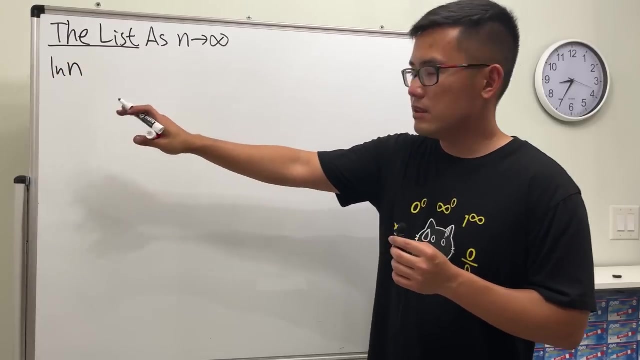 the factorial with us and then, um, it doesn't really matter, of course. you can use t, you can use x, doesn't matter. here we go among all the functions that go to infinity: l, n or any kind of log, any kind of law functions. it's a small list, so small that i'm going to put two less. 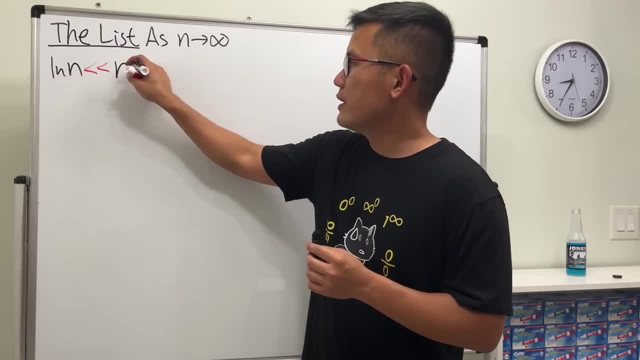 than symbols like this, and then you're going to put two less than symbols like this, and then you're going to put two less than symbols like this, and then you're will see why. next we have n to the power, like a power function or power sequence. 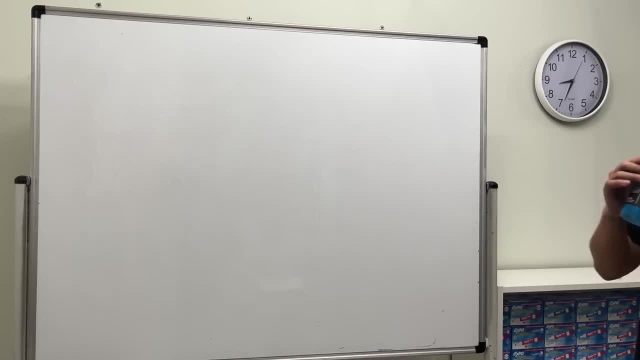 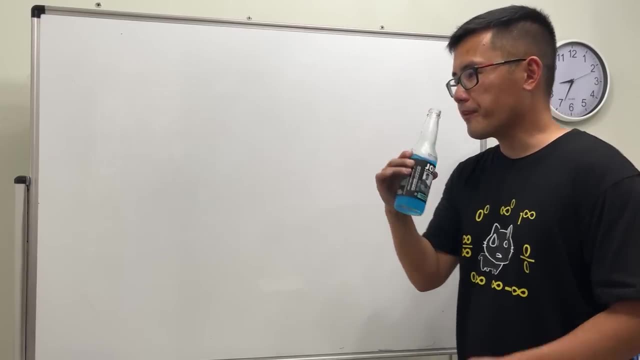 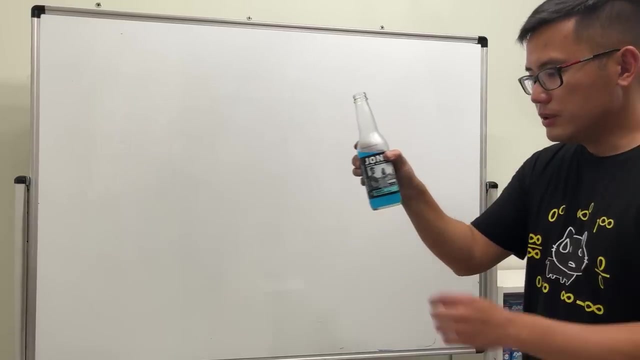 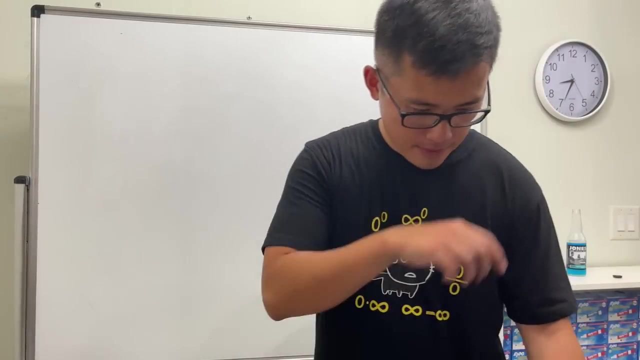 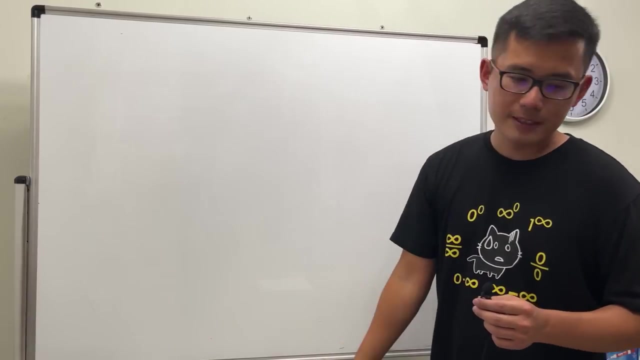 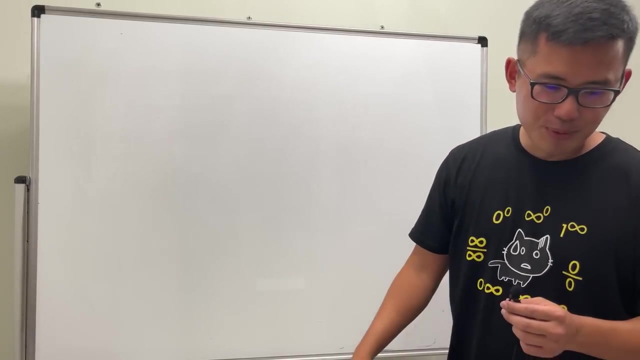 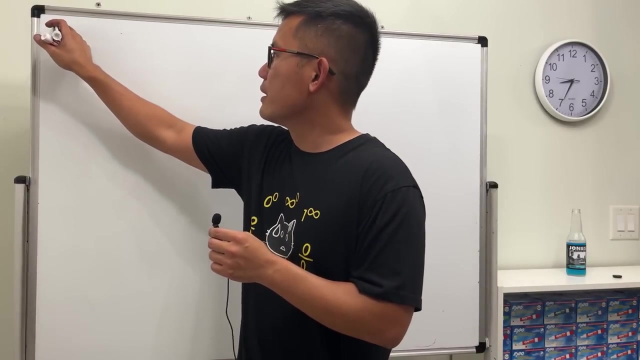 Oh, it says real, but nothing said by real. Anyway, I should have bought some Gatorade. I forgot It's hot. Yeah, that's why I have to drink something. But anyway, though, 30 more questions. Secret weapon number one: I call this the list. 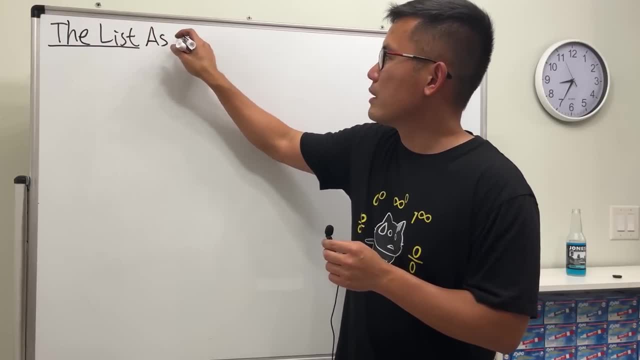 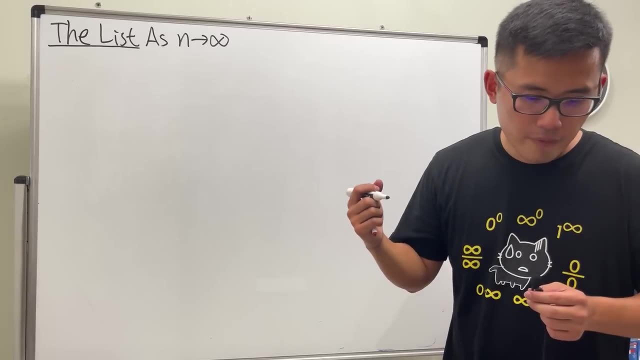 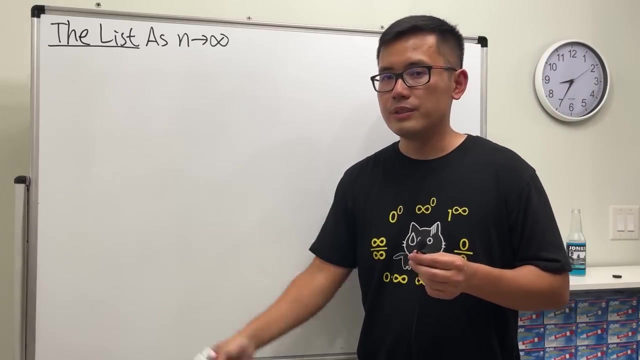 What's the list? Well, this is to compare the kind of infinities. I'm using n right here, because this way I can also bring the factorial with us, And then it doesn't really matter. Of course, you can use t, you can use x. 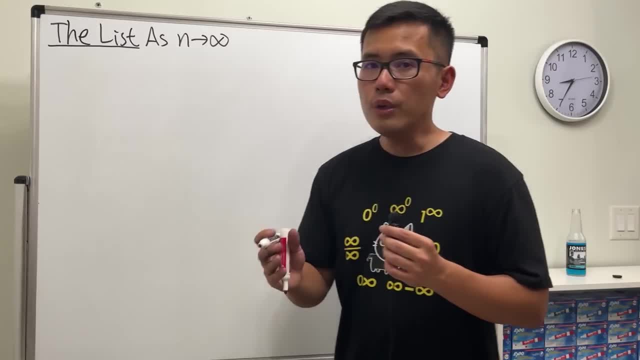 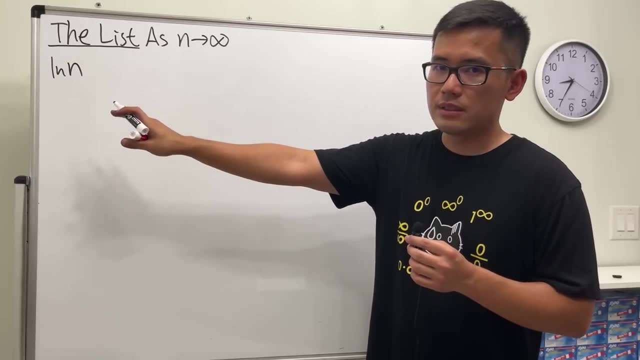 Doesn't matter. Here we go. Among all the functions that go to infinity, ln or any kind of log, any kind of log functions, it's the smallest. So small that I'm going to put two less than symbols like this, and then you will see why. 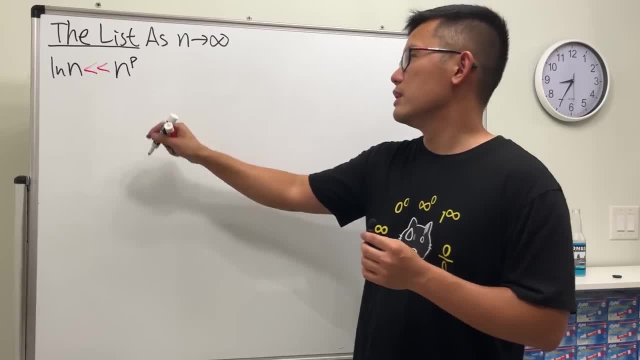 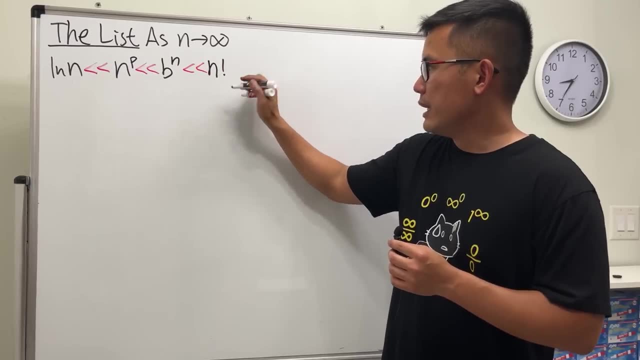 Next we have n to the power, like a power function or a power sequence, But anyway, though, continue. Next we have b to the n, And next here is the factorial, And then next the biggest one, n to the n. 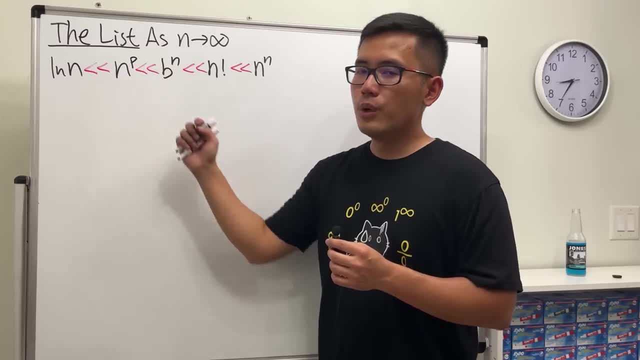 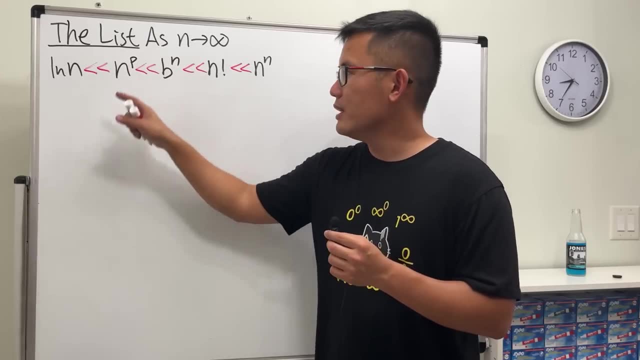 Power tower. However, in order for this to go to infinity- well, you see, n goes to infinity right, And we talked about this earlier, like two, three hours ago- The power right here has to be positive. So let me just indicate that. 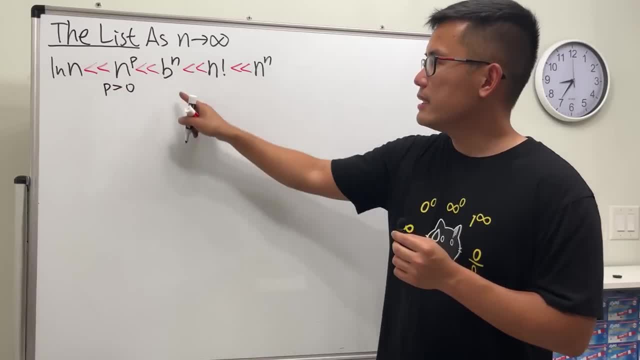 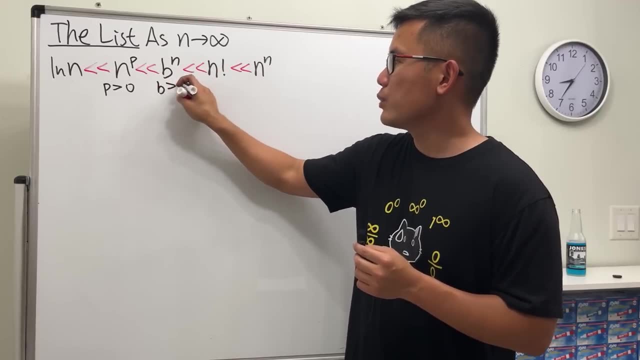 p has to be positive, So it has to be greater than zero here. And then, in order for exponential to go to infinity, the base has to be greater than one, So p has to be greater than one. So this right here is the list. 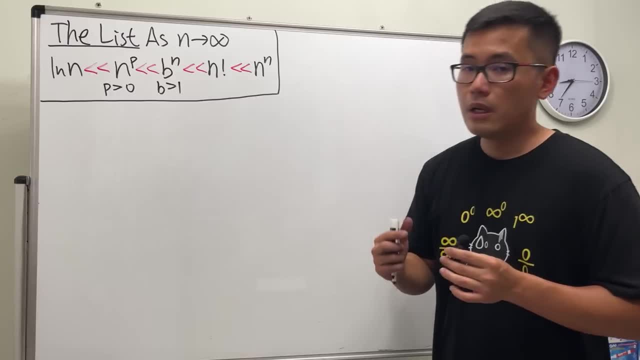 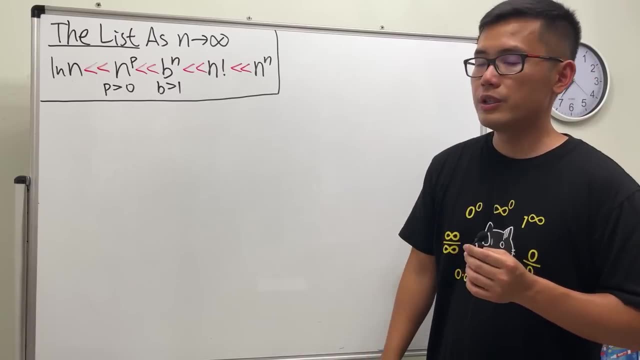 If you know it, you can solve a lot of limit equations in no time. I tell my students that you can just tell me what the answers are. if the limits fit into this situation, How do we use it? Let me show you Number 72.. 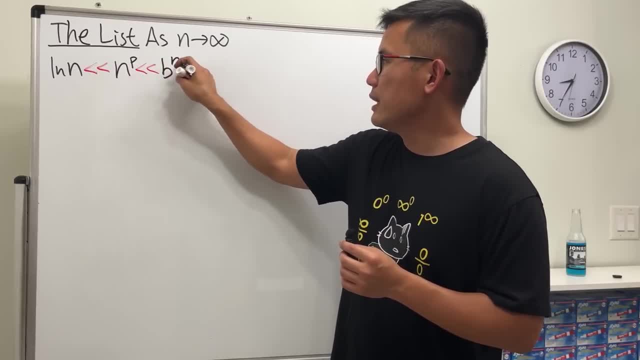 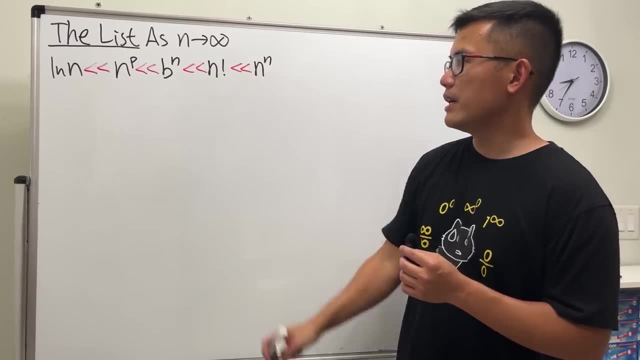 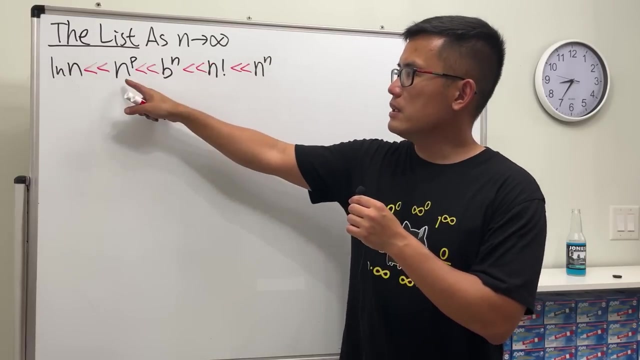 but anyway, though, continue. next we have b to the end, and next here is the factorial, and then next the biggest one, n to the n power tower. however, in order for this to go to infinity, well, you see, n goes to infinity right, and we talked about this earlier. 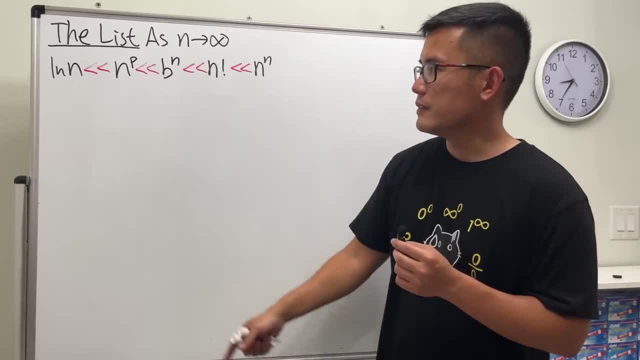 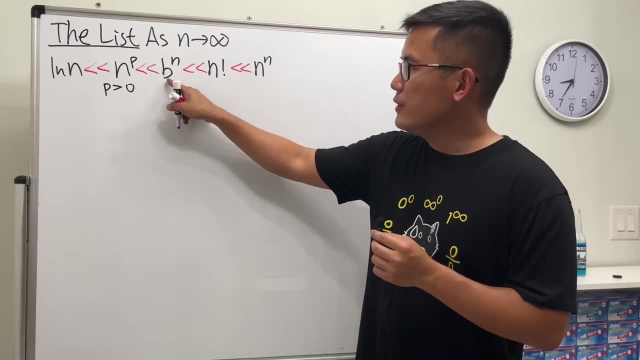 like two, three hours ago. the power right here has to be positive. so Let me just indicate that p has to be greater than 0 here, And then, in order for exponential to go to infinity, the base has to be greater than 1.. So p has to be greater than 1.. 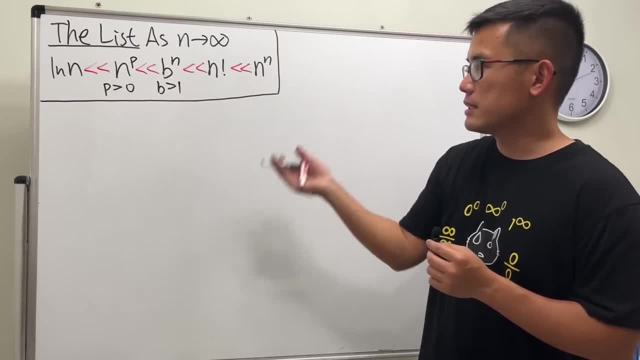 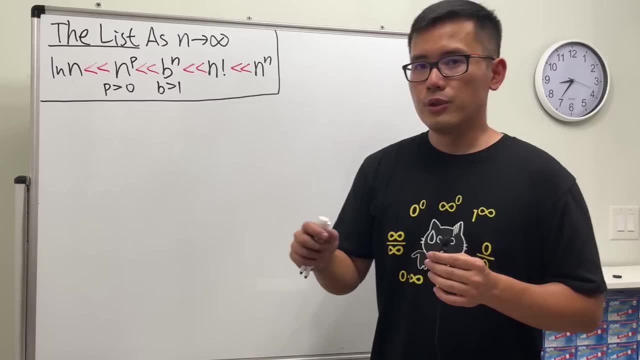 So this right here is the list. If you know it, you can solve a lot of limit equations in no time. I tell my students that you can just tell me what the answers are. if the limits fit into this situation, How do we use it? 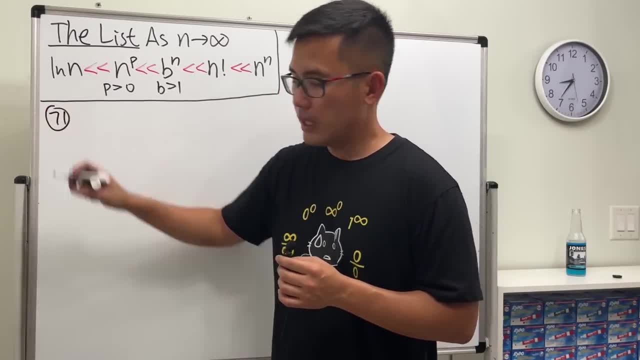 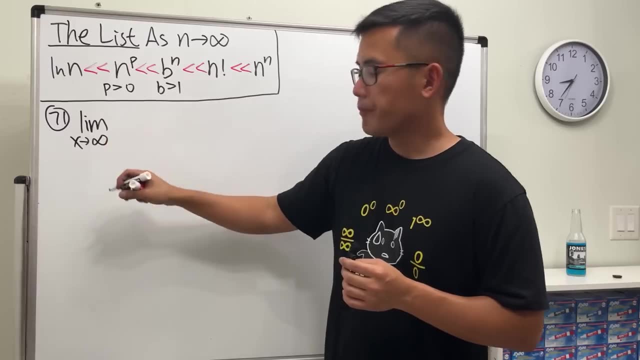 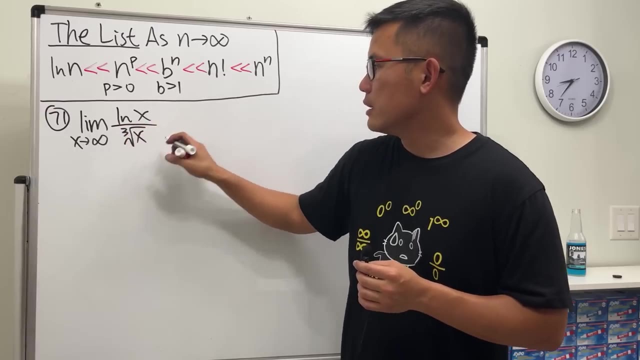 Let me show you Number 71. I'm going to give you guys two questions. If today we have the limit as x approaching infinity, and then we have ln x over the cube root of x, Well, ln x is a small kind of infinity. 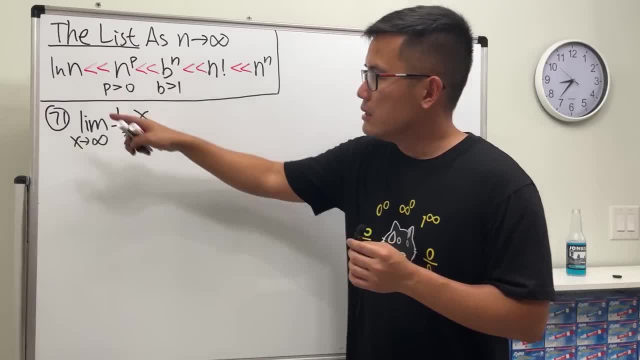 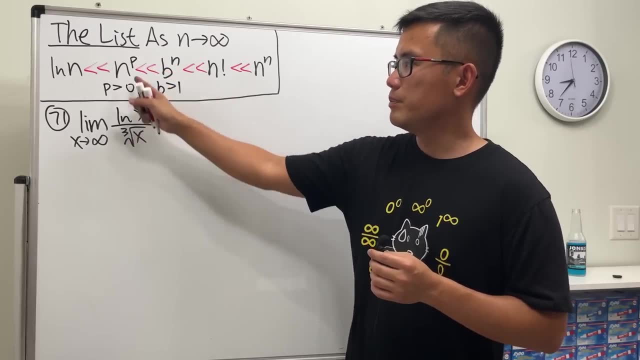 And the reason I put down 2 less than simple is that this is so small, Such that when you do the ratio, if you have small over something that's bigger- because this is the same as x to the 1 third power which belongs to here. 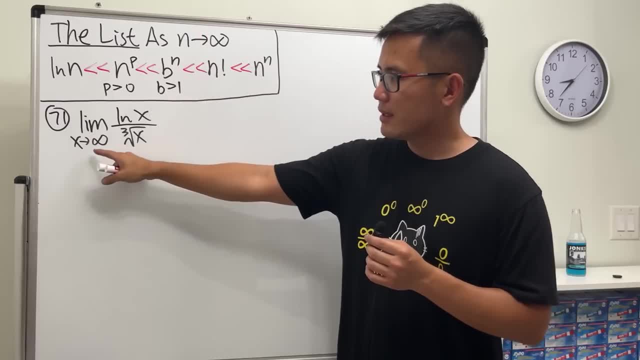 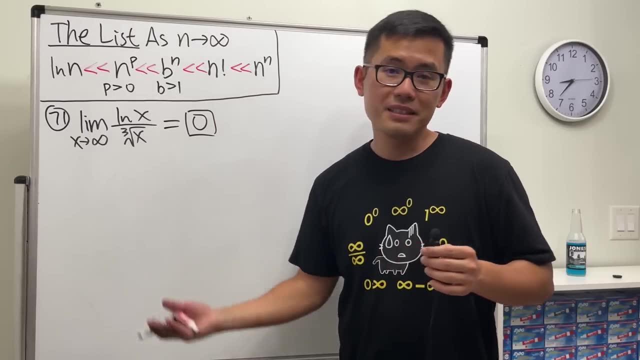 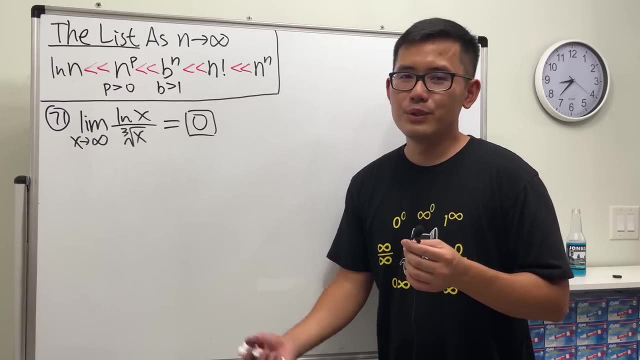 When you divide them and take the limit, as x goes to infinity, let me tell you the answer is just equal to 0.. Yeah, Yes, that's it. That's it For my students. you can say the list If you don't quote the. 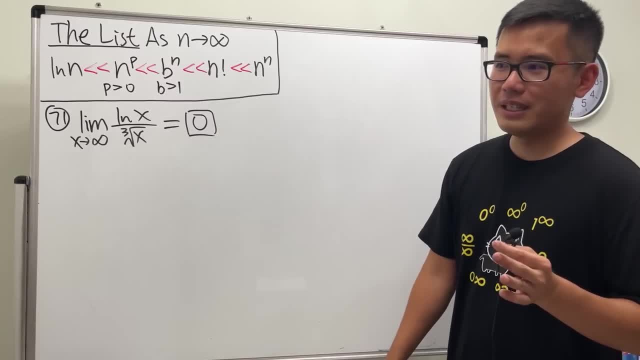 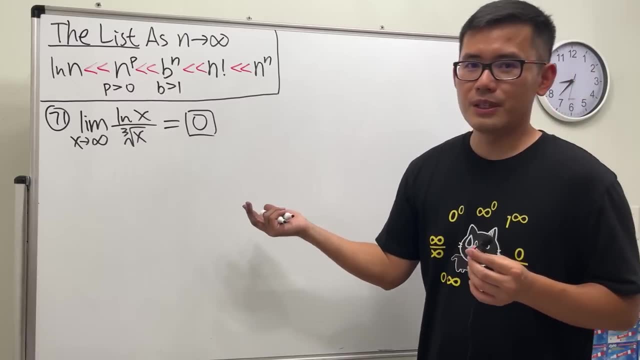 Grease and nuts. Fine too, But if you're not my student, if you are taking your calculus 2 class, then do not say this is equal to 0 by the list. Your professor is not going to understand what you are talking about. 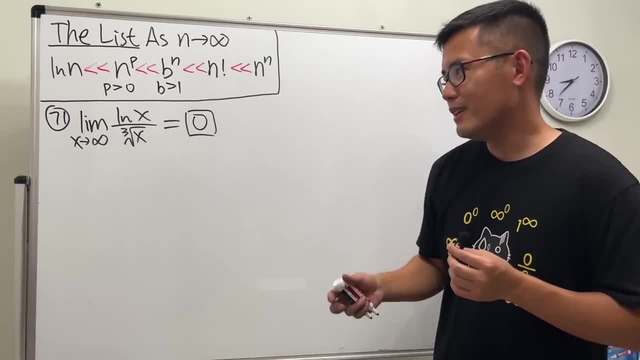 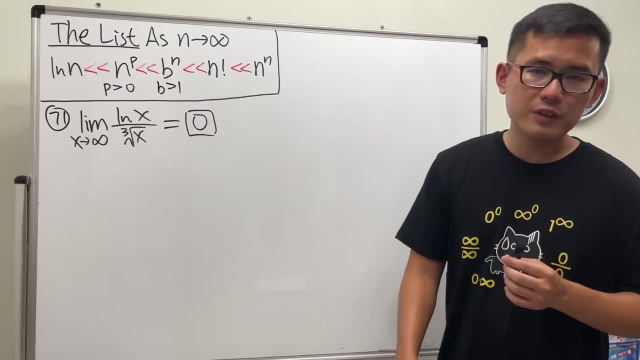 So yeah, By the way, this is just that you can keep in mind. So it's a magic: When you see this kind of limit, you can put down 0 right away. The proof for this is to use L'Hopital's rule, which is very similar to number 70.. 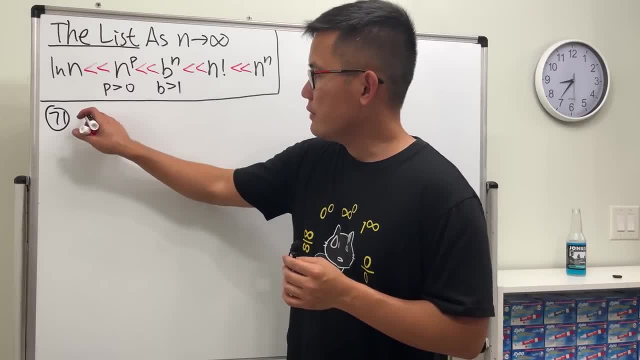 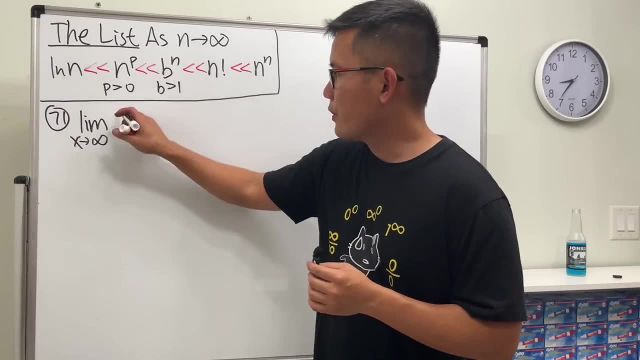 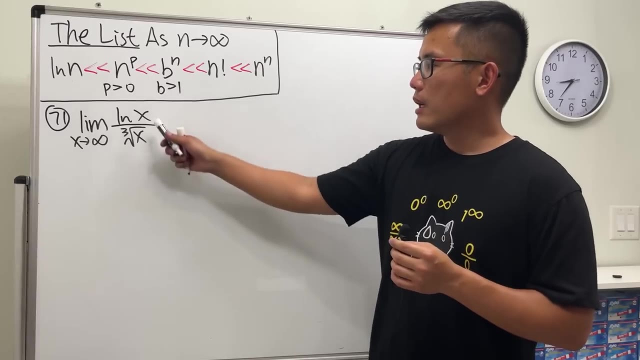 One. I'm going to give you guys two questions. If today we have the limit as x approaching infinity, and then we have ln x over the cube root of x, Okay Well, ln x, it's a small kind of infinity. 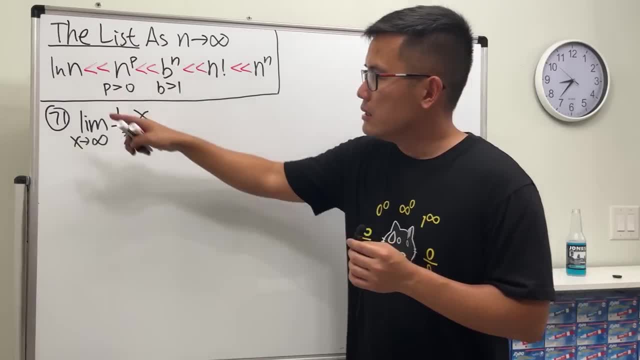 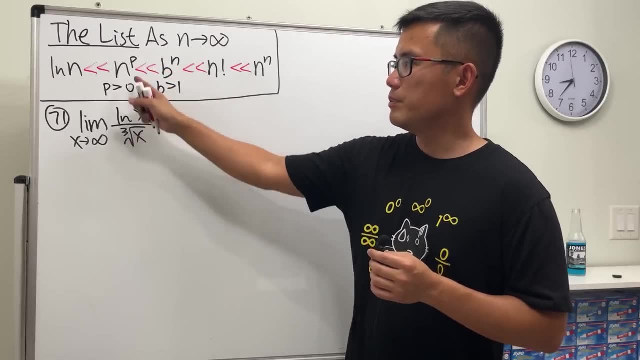 Yeah, And the reason I put down two less than symbols is that this is so small, such that when you do the ratio, if you have small over something that's bigger, because this is the same as x to the one-third power which belongs to here. 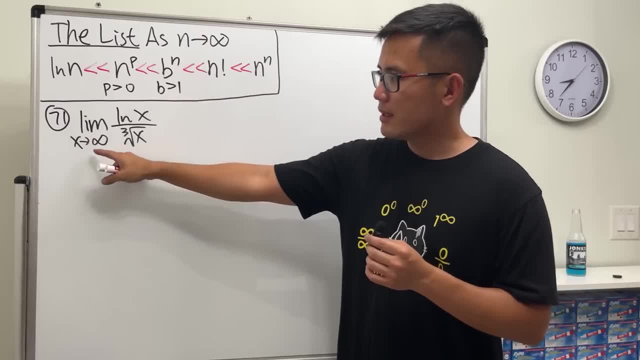 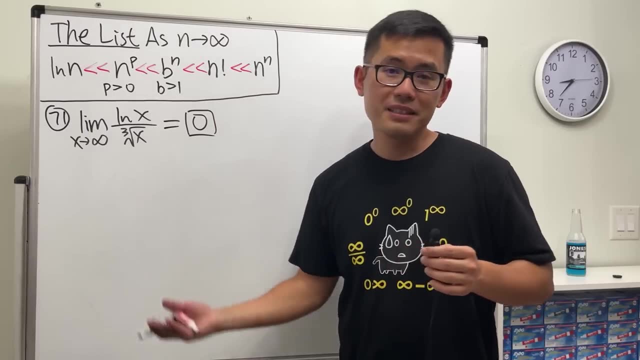 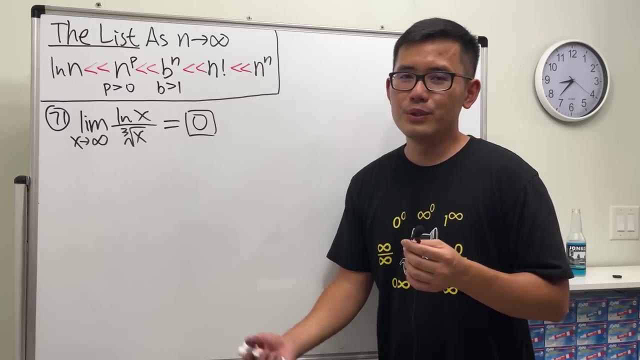 when you divide them and take the limit, as x goes to infinity, let me tell you the answer is just equal to zero. Yeah, Yes, that's it. That's it For my students. you can say the list. If you don't quote the reason, that's fine too. 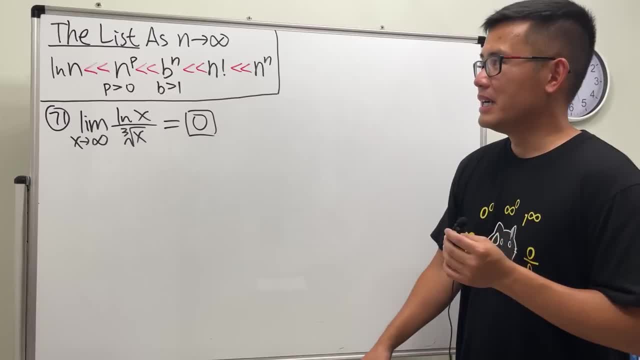 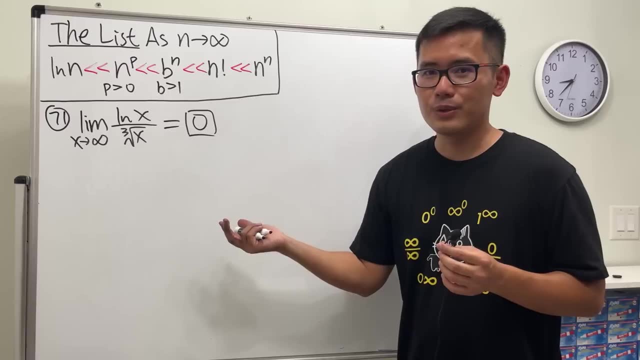 But if you're not my student, if you are taking your calculus two class, then do not say this is equal to zero by the list. Your professor is not going to understand what you are talking about. So yeah, By the way, this is just that you can keep in mind. 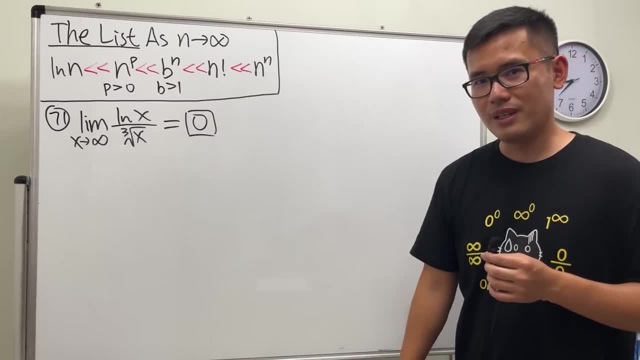 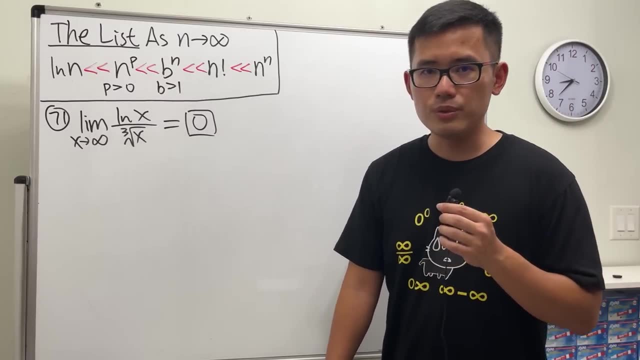 So it's a magic When you see this kind of limit, you can put down zero right away. The proof of this is to use L'Hopital's rule, which is very similar to number 70.. That's why I told you guys to pay attention to the question earlier. 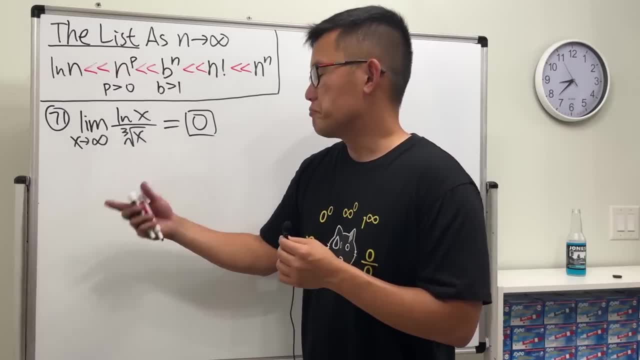 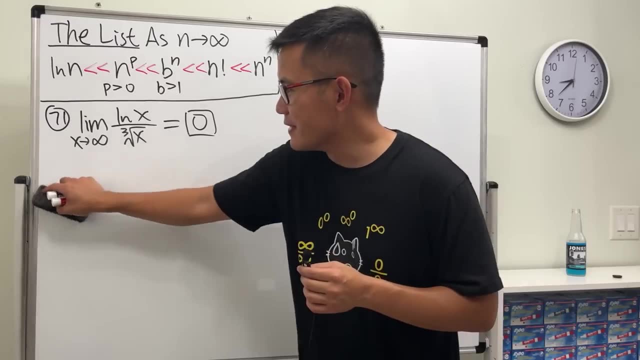 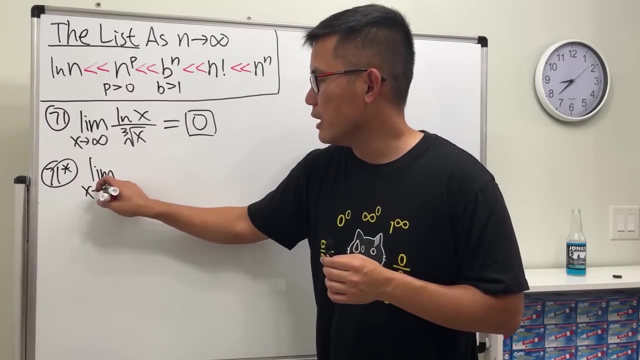 All right, Okay, So this is that. But what if like this is just first, this is like versus. So I'm going to put it as 71 star to make it slightly more clear. But what if we have the question being the limit as x approaching infinity? 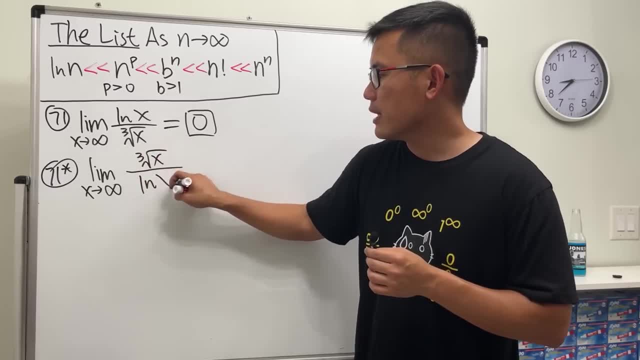 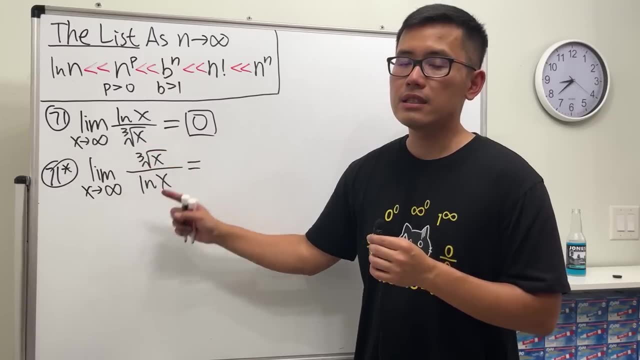 We have the cube root of x on the top and then Lnx on the bottom. Well, you can read it backwards: This right here is so big compared to that, Big enough So that when you look at it, if you divide them and then take the limit as x goes to infinity. 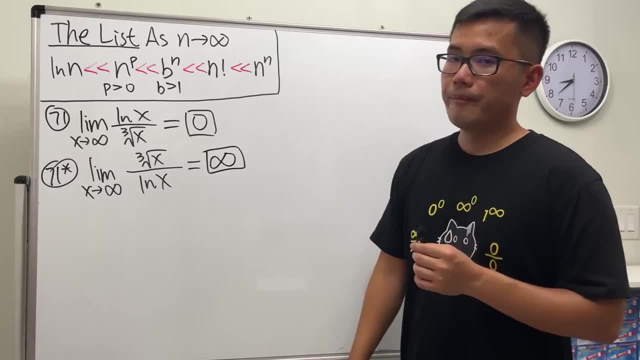 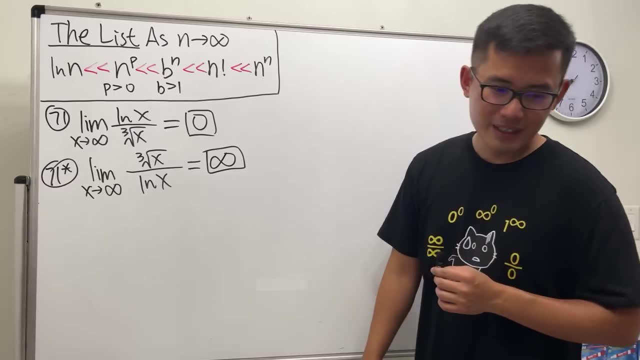 you get infinity. Yeah, So when you're comparing this kind of functions with sequence, either you get zero or infinity. when you're using the list, So cool. So we will have a lot of questions that we can actually just finish in no time. 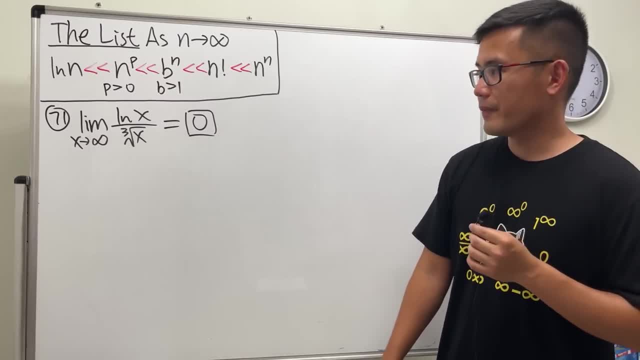 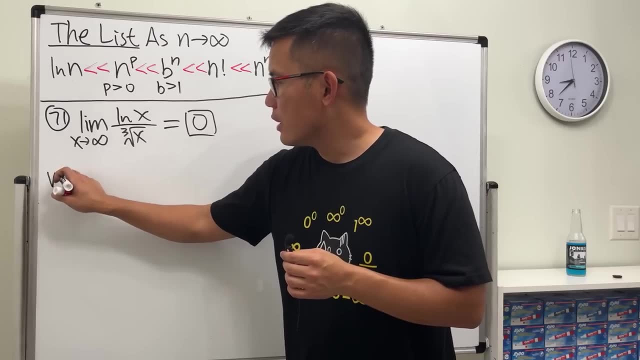 That's why I told you guys to pay attention to the question earlier. All right, Okay, So this is that. But what if? Now? this is just first? This is like firsts, So I'm going to put it as 71 star to make it slightly more clear. 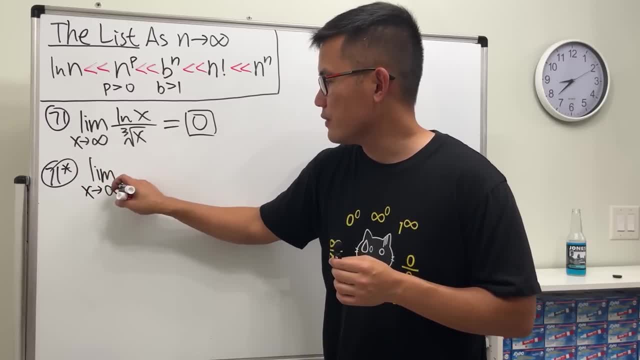 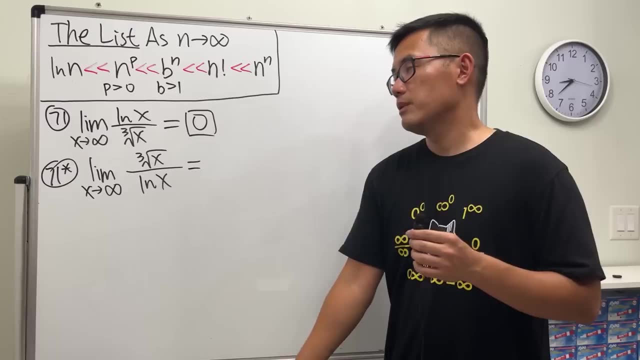 But what if we have the question being the limit as x approaching infinity? we have the cube root of x on the top and then Lnx on the bottom. Well, you can read it backwards: This right here is so big compared to that. 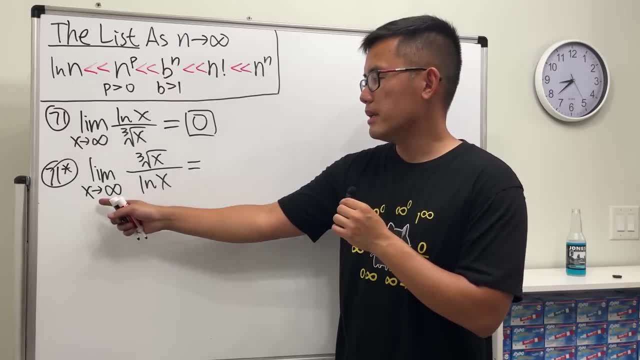 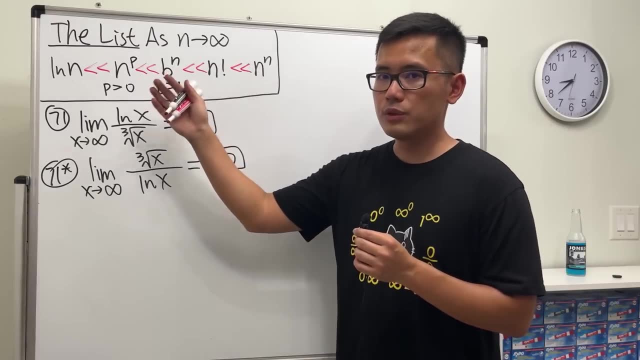 Big enough So that when you divide, Divide them and then take the limit, as x goes to infinity, you get infinity. Yeah, So when you're computing this kind of functions or sequence, either you get 0 or infinity. when you're using the list, 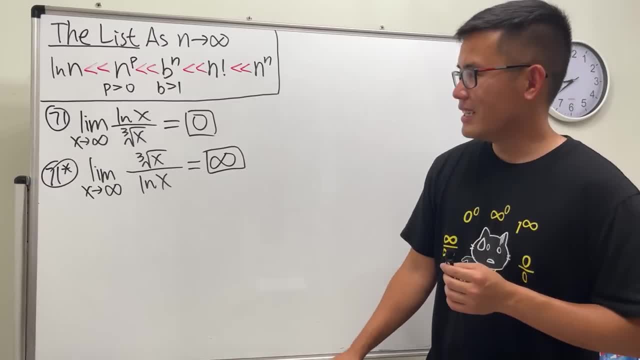 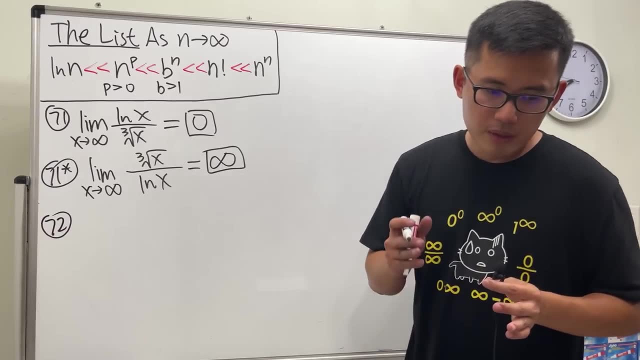 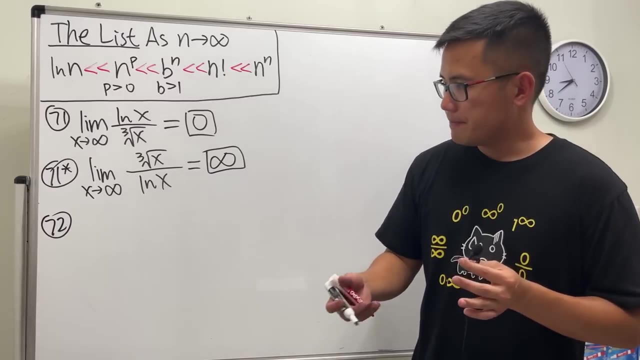 So cool, So we will have a lot of questions that we can actually just finish in no time, By the way, number 72.. Number 72 tells you the. The purpose of number 72 is to show you the How to pick out the dominating part. 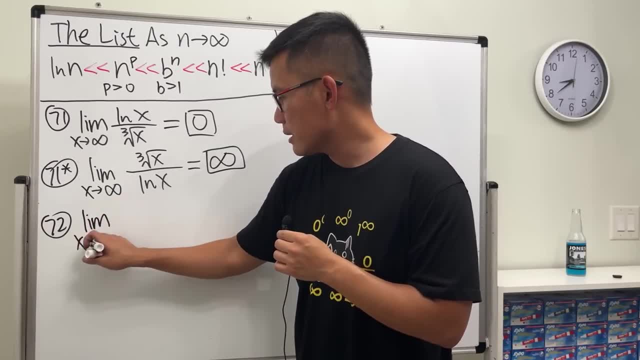 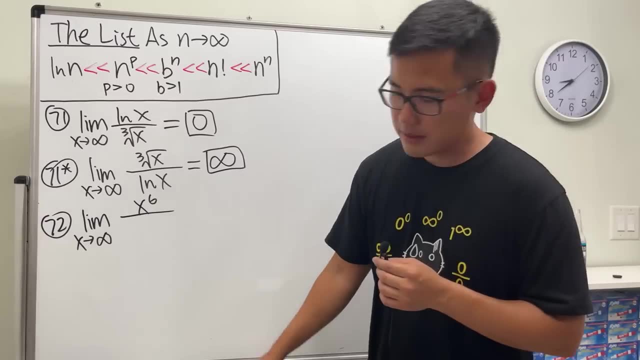 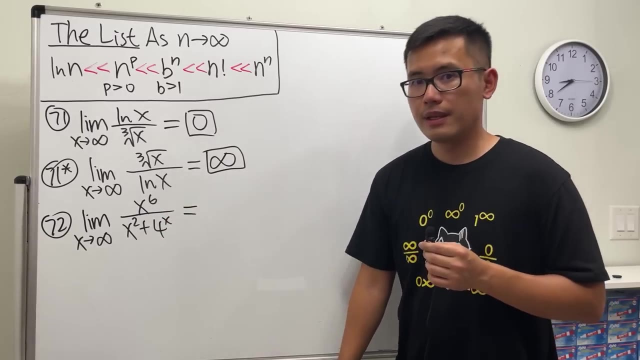 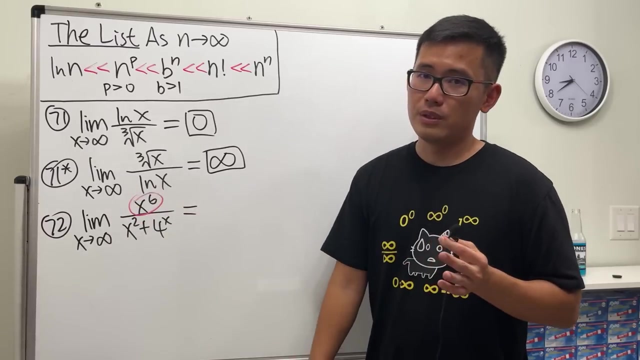 But anyway, let's see Number 72, we have the limit as x approaching infinity, and then we have x to the 6th power over x squared plus 4 to the x. Okay, On the top we have x to the 6th power. 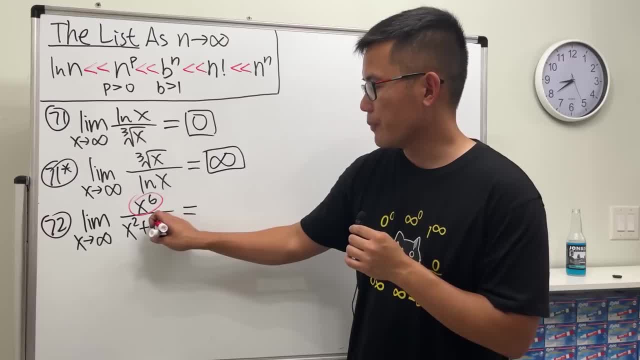 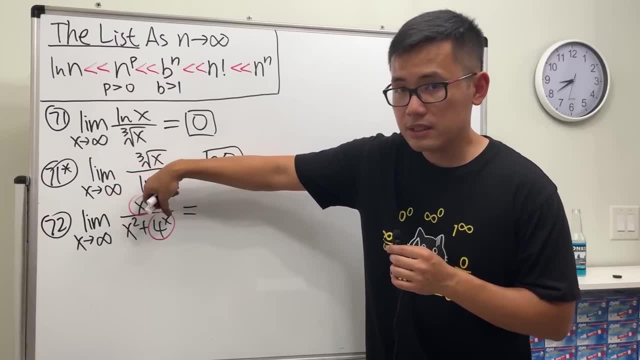 Okay, On the bottom we have 4 to the x. So look at this, Don't look at that. Why? Because if you compare the bottom x squared versus 4 to the x, 4 to the x is bigger. 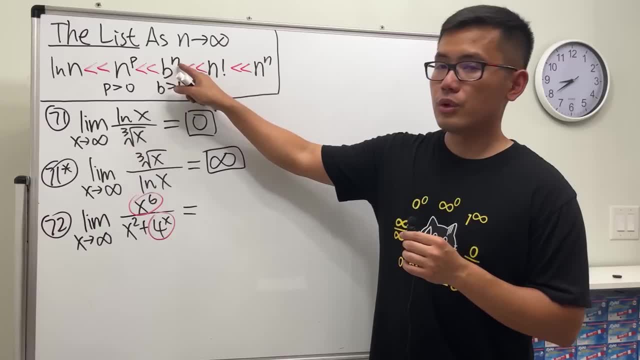 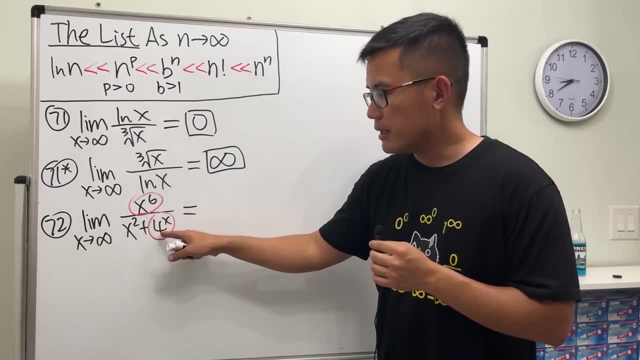 It's dominating. It's the exponential part, Right A number to the exponent power. Right x will end Yeah. And now if you compare this and that, 4 to the x is bigger but it's on the bottom. 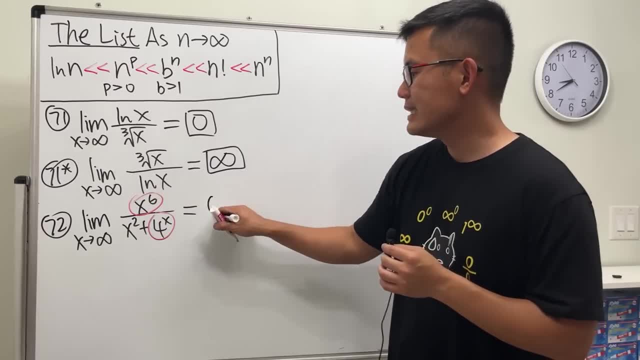 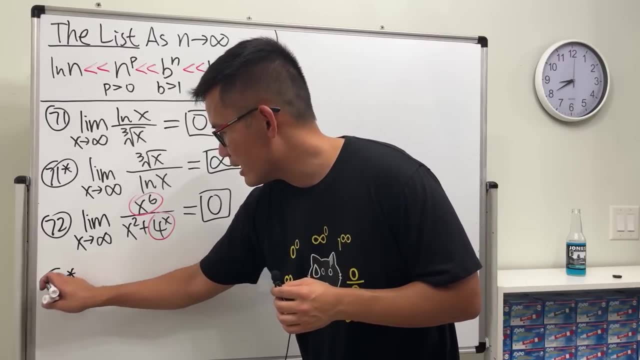 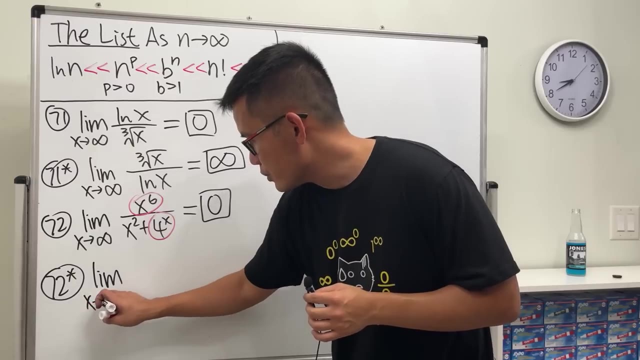 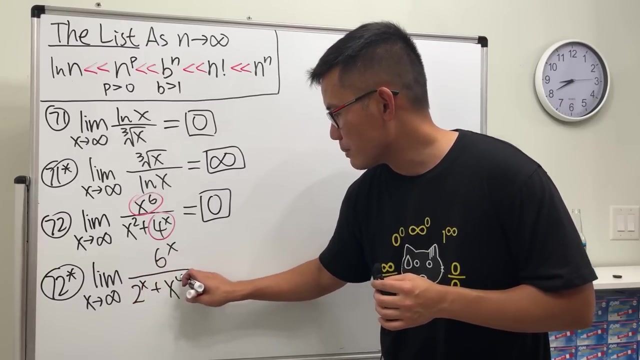 So that means when we do the limit of this we get 0. Done 72 star. If I change this a little bit, if I change this to the limit as x approaching infinity, 6 to the x power and then 2 to the x and then x to the 4th power. 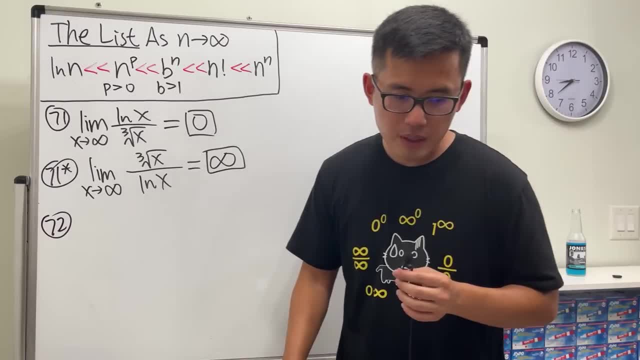 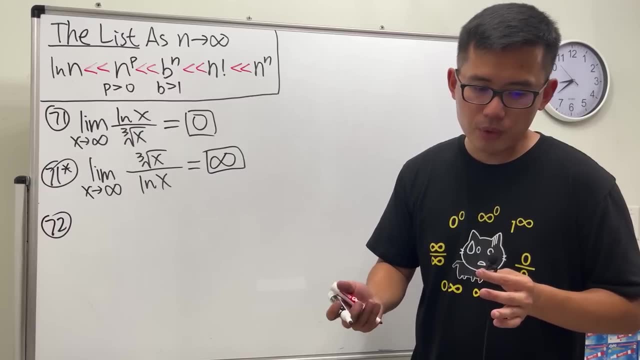 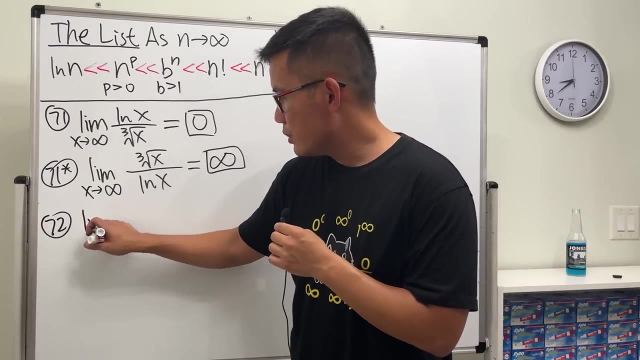 By the way, number 72.. Number 72 tells you the. the purpose of number 72 is to show you the how to pick out the dominating part. But anyway, let's see Number 72,. we have the limit as x approaching infinity. 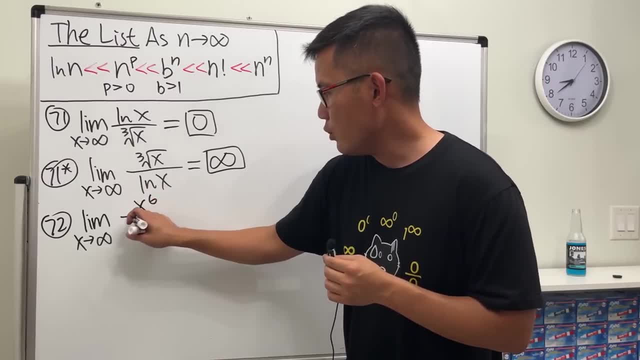 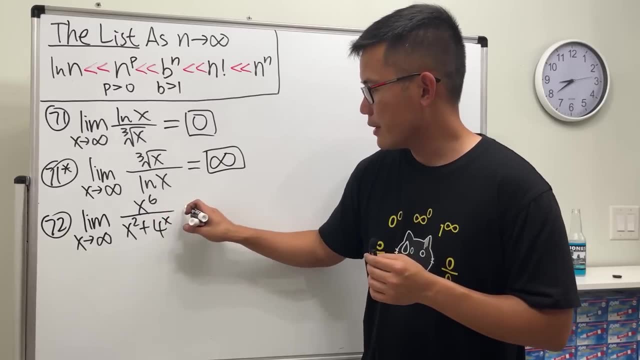 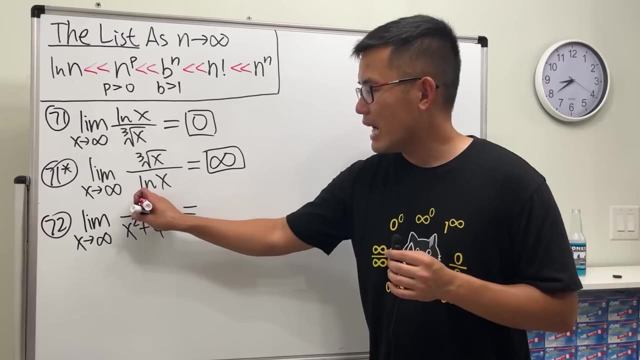 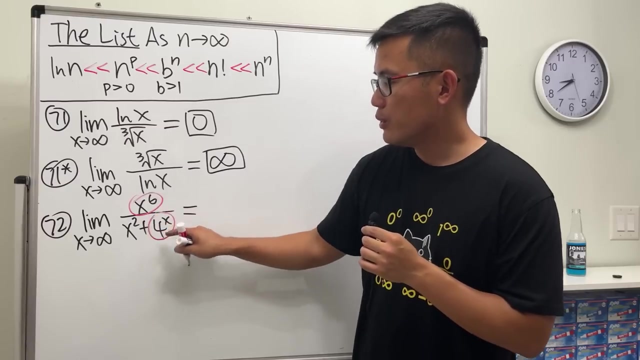 And then we have x to the sixth power over x square, plus four to the x. Okay, On the top we have x to the sixth power. Okay, On the bottom we have four to the x. So look at this, Don't look at that. 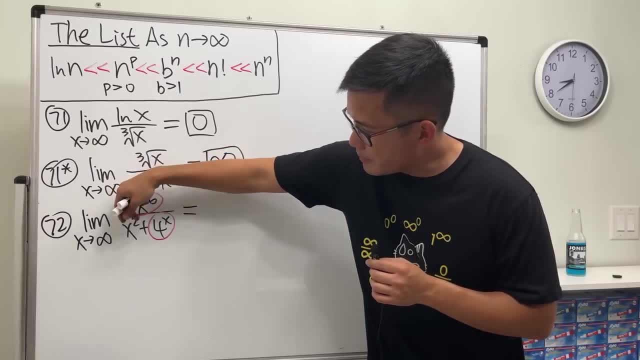 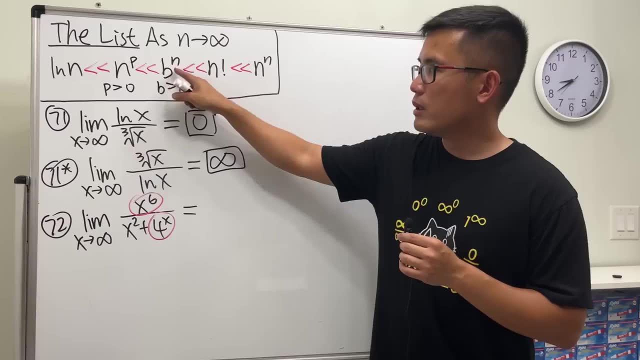 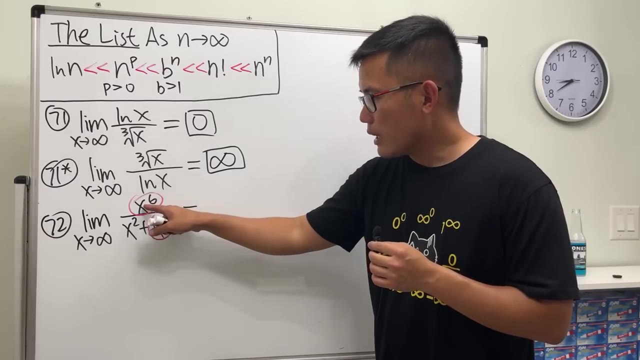 Why? Because if you compare the bottom x square versus four to the x, four to the x is bigger, It's dominating, It's the exponential part, right A number to the exponent power, right, X will end Yeah. And now, if you compare this and that, 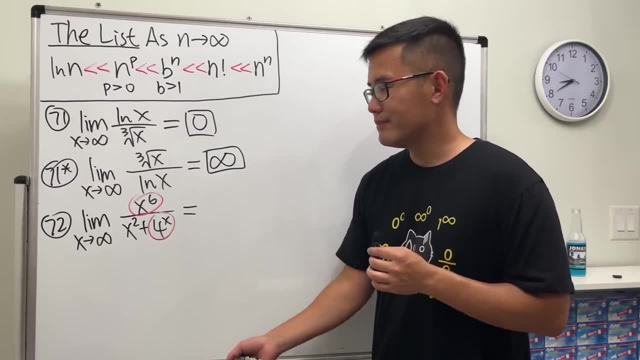 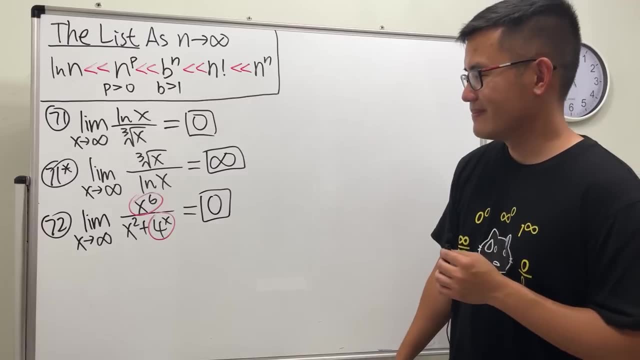 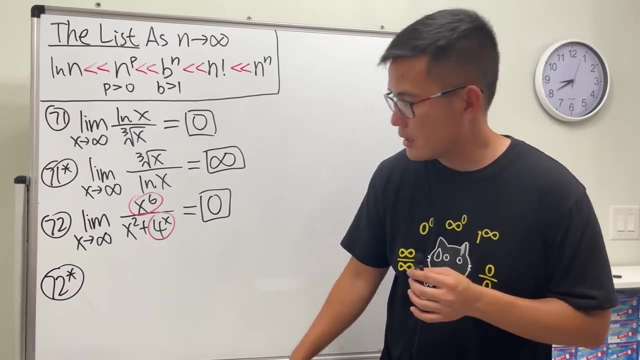 four to the x is bigger but it's on the bottom. So that means when we do the limit of this we get zero. Done 72, star. If I change this a little bit, if I change this to the limit as x approaching infinity. 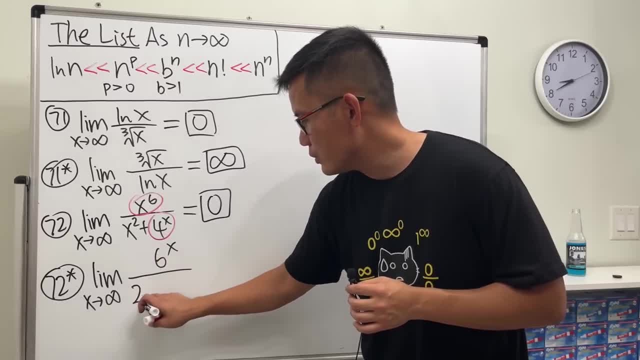 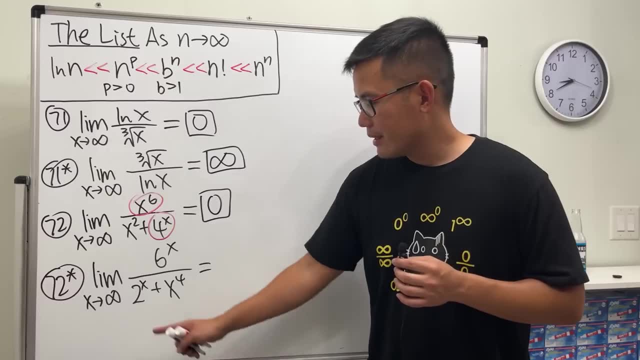 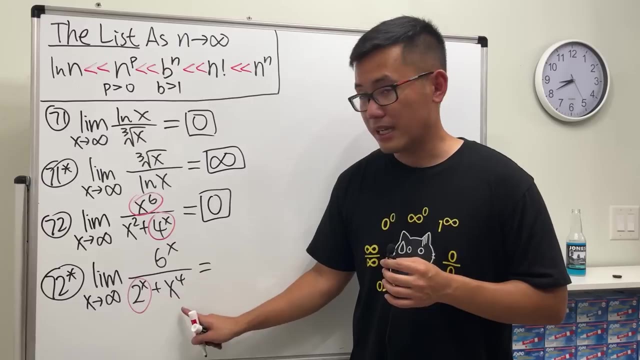 six to the x power and then two to the x and then x to the fourth power. What do you think? what the answer is? Compare the bottom two to the x versus x to the four. This time two to the x is bigger than that. 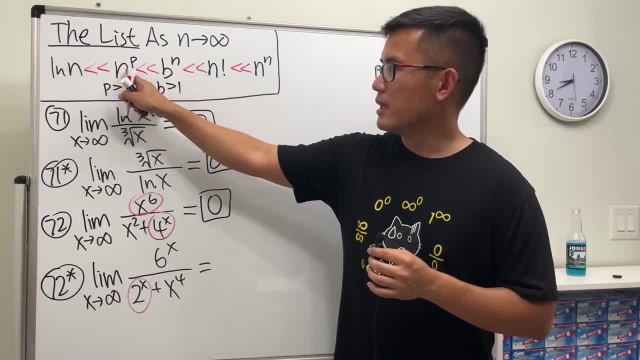 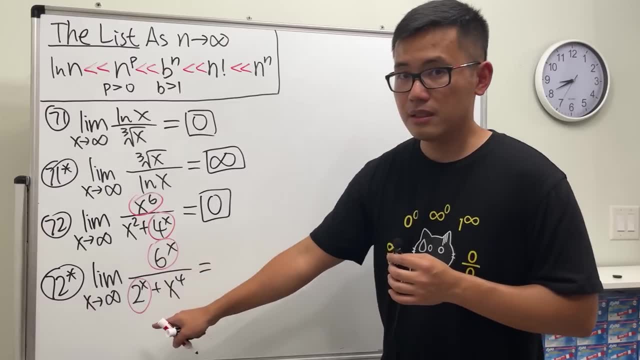 It dominates the exponential part, It dominates the x to the p right, So x to the fourth, And then if you compare this and that, well, the top is bigger than that. Even they are in the same category. So of course you look at which bigger 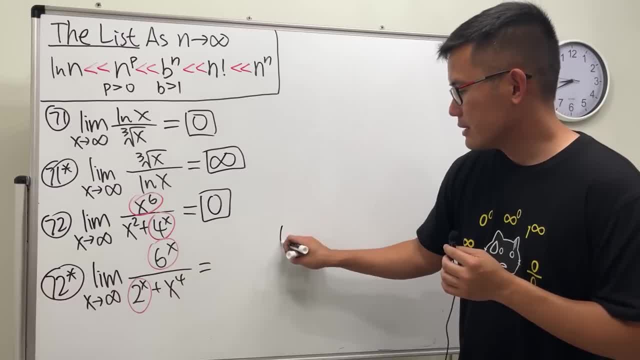 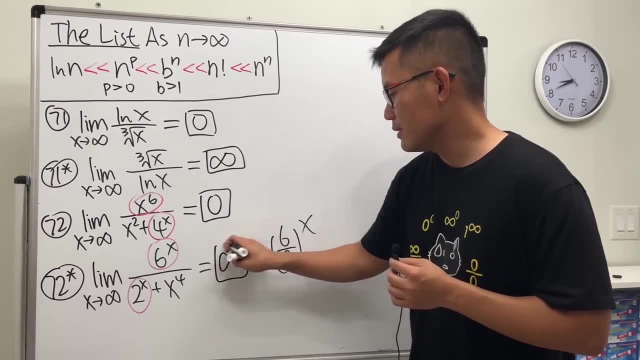 which base is bigger, And you can actually just see this as six over two to the x power, And then it's just three to the x power When x goes to infinity is infinity. But yeah, that's it, That's how you do it. 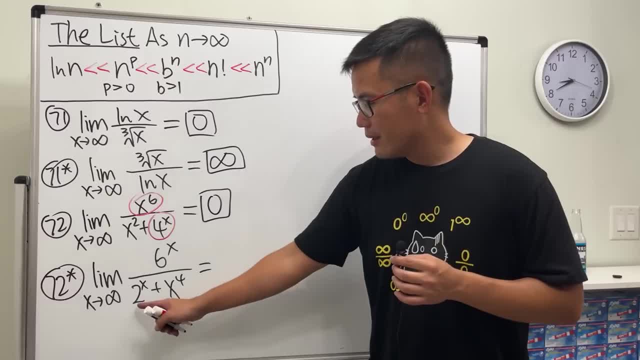 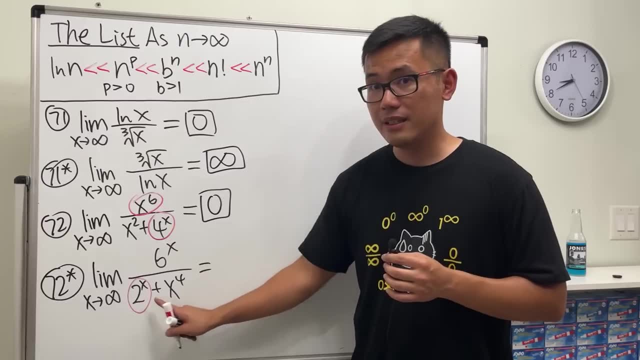 What do you think? what the answer is. Compare the bottom 2 to the x versus x to the 4. This time, 2.. 2 to the x is bigger than that. It dominates the exponential part. It dominates the x to the p. 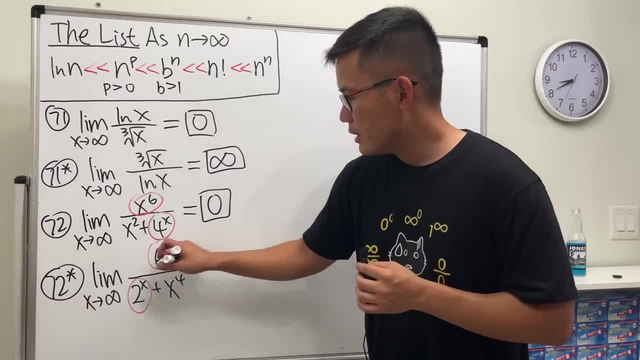 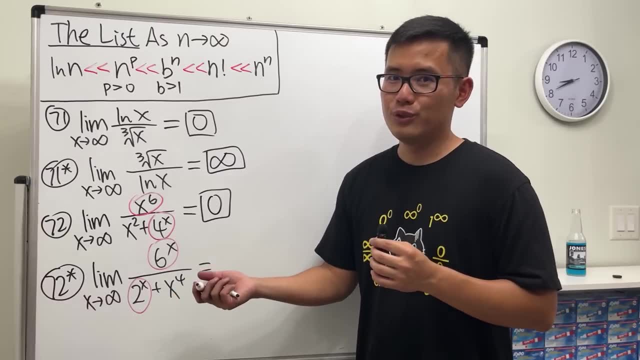 So x to the 4th And then if you compare this and that, well the top is bigger than that. Even they are in the same category. So of course you look at which base is bigger And you can actually just see this as 6 over 2 to the x power. 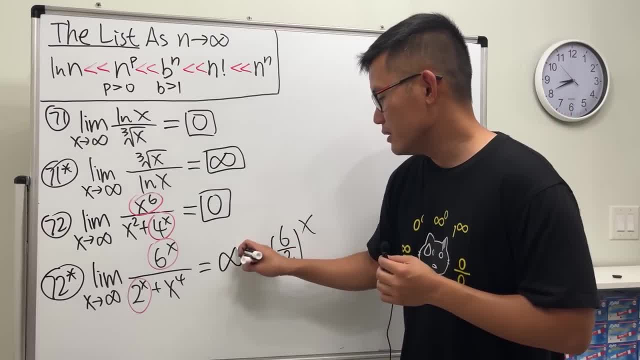 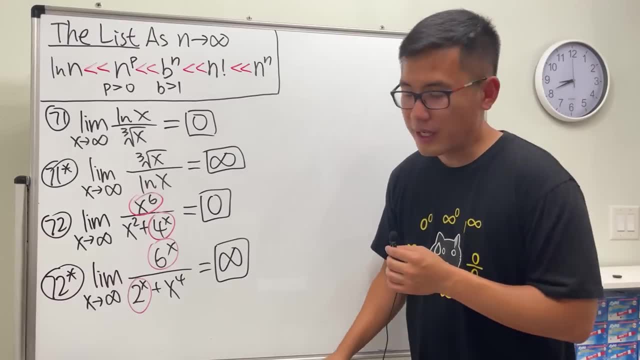 And then it's just 3 to the x power. When x goes to infinity, it's infinity. But yeah, that's it. That's how you do it. Okay, number 73.. Oh man, this is the last question. 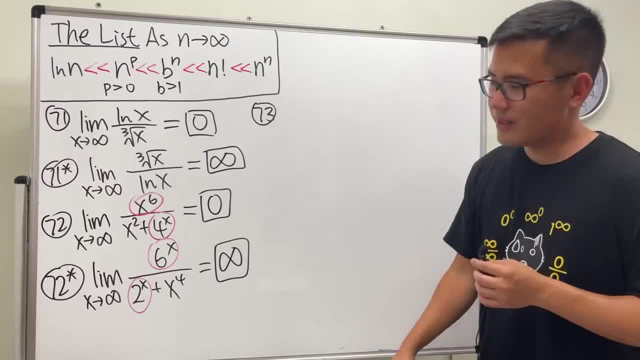 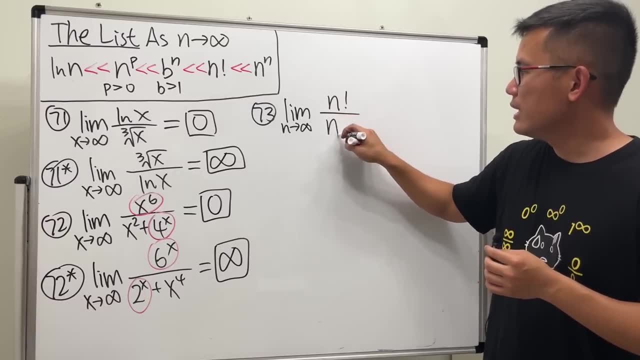 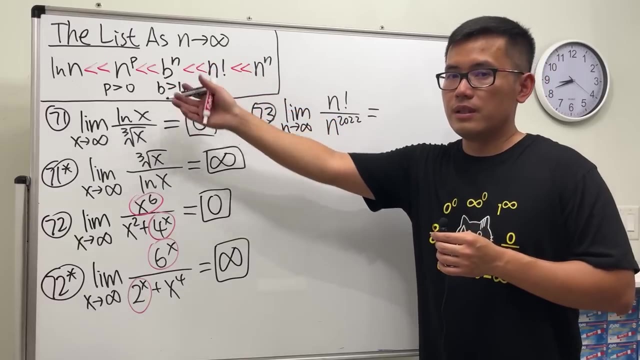 No, I have a couple more for the list. I have 5 questions for the list. I like that Limit as n goes to infinity, n factorial over n to the 20, 22.. And this is the reason why I put n to be the list right for the list. 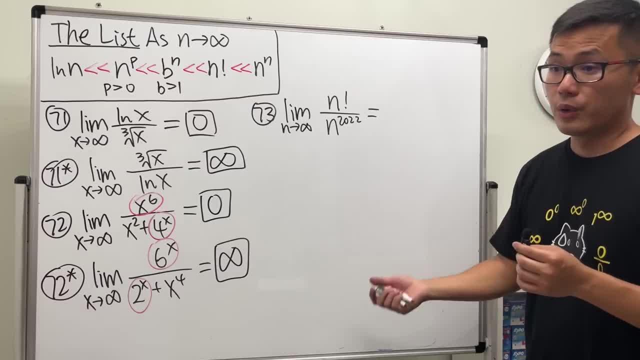 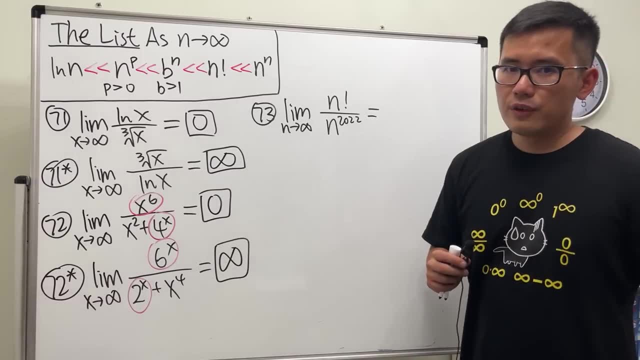 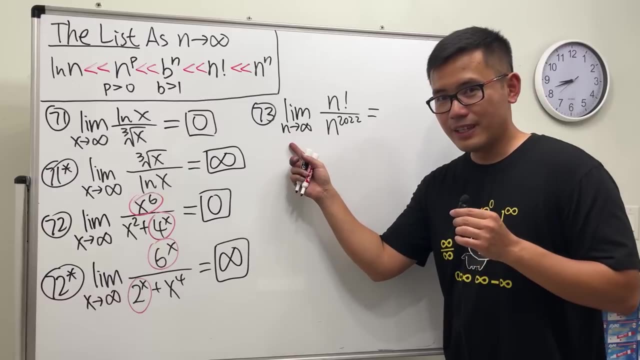 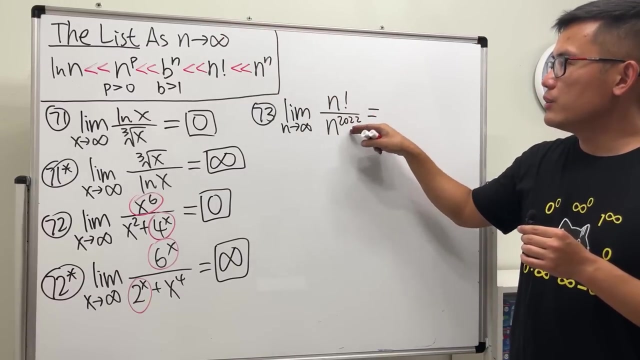 Because that's how we can say n factorial, for positive odd number factorial or maybe 0 factorial, You can do like fractional factorial, but that's a different story. That will be later on, not now. Anyway, when n goes to infinity, n factorial is so much bigger than n to the p's power, right? 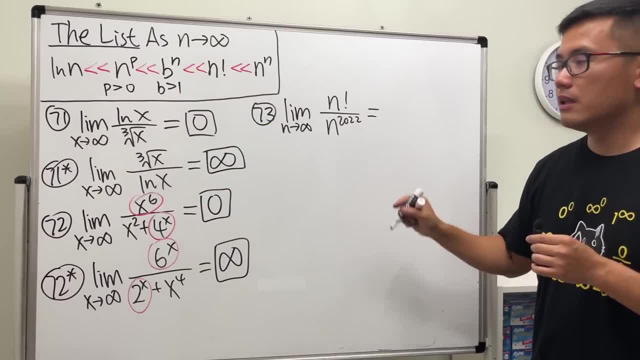 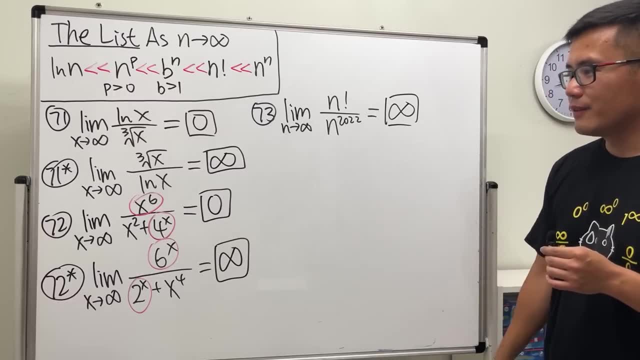 n to the power. So this is bigger than that. Therefore, the answer is: what Infinity Done? You can give me 1,000 of these questions. I can finish it. I don't know, I don't want to do it actually. 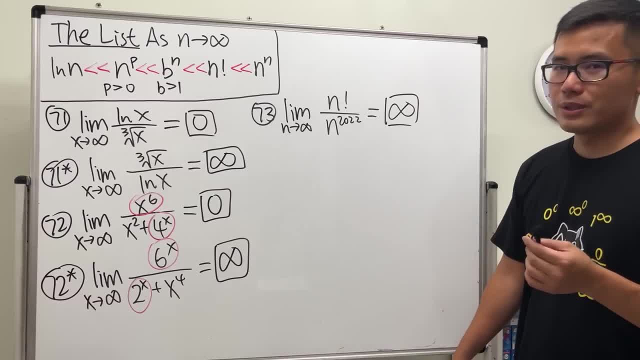 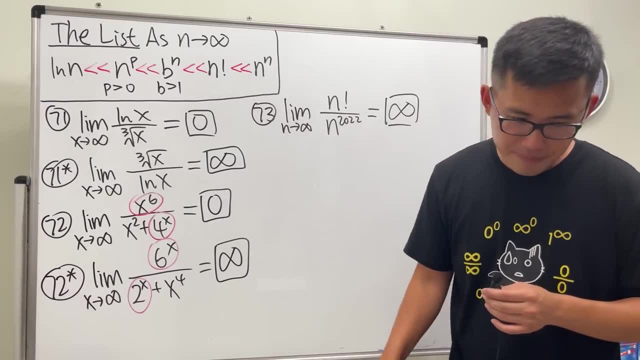 You can give me 100 of these questions. I can do it in like 2 hours or 1 hour, maybe, By the way, 10 seconds, I don't know. Okay, next 74.. If we have the limit as n goes to infinity. 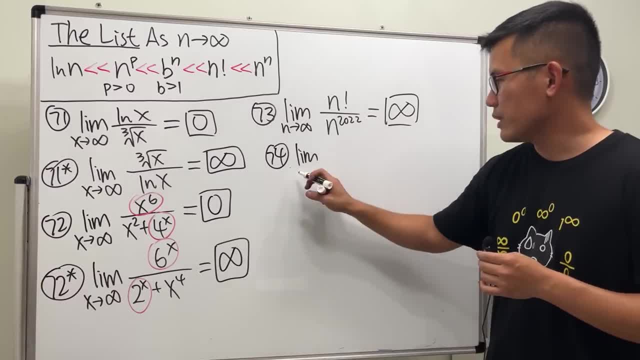 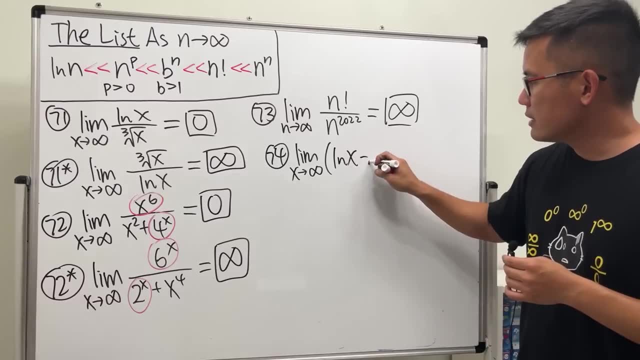 No, I use x Most of the time. we are talking about x. x is much better because we can do L'Hopital's rule. It's like ddx and all that stuff. But anyway, Lnx minus square root of x. 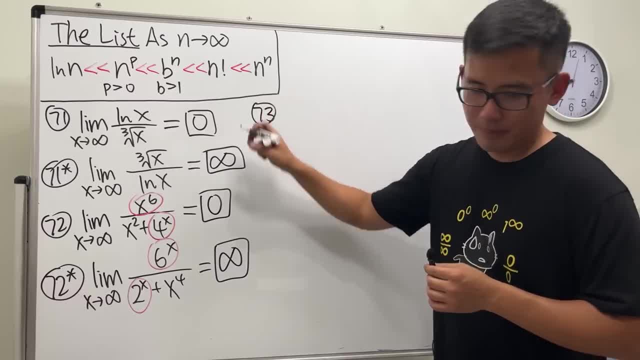 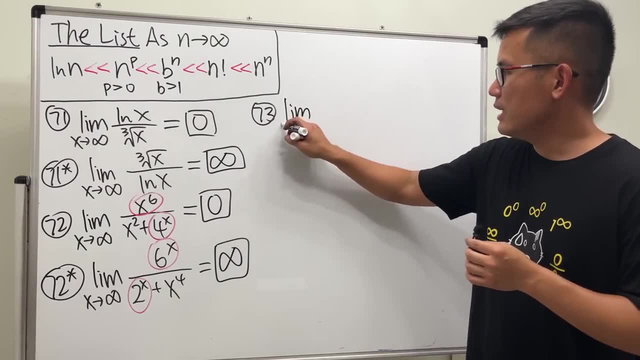 Okay, Number 73.. Oh man, this is the last question. No, I have a couple more for the list. I have five questions for the list. I like that Limit as n goes to infinity and factorial over n to the 2022.. 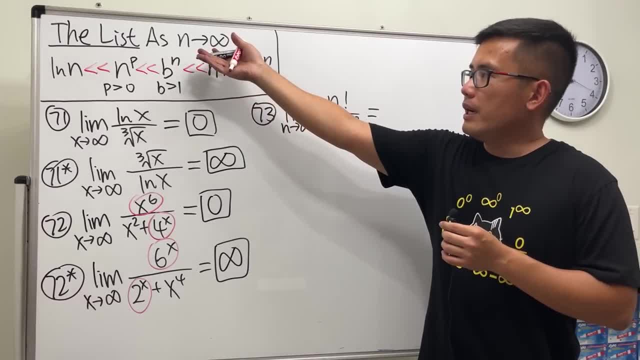 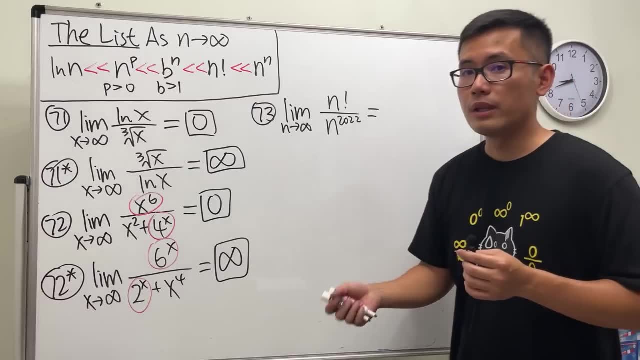 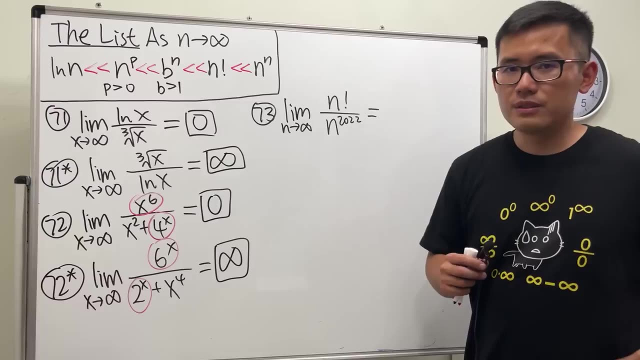 And this is the reason why I I put n to be the list, right for the list, because that's how we can say n factorial for positive whole number factorial or maybe zero factorial. You can do like fractional factorial, but that's a different story. 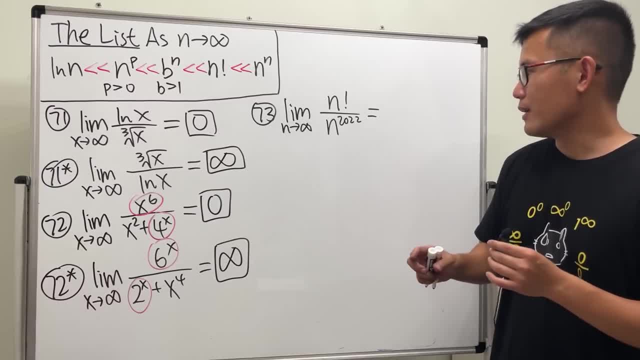 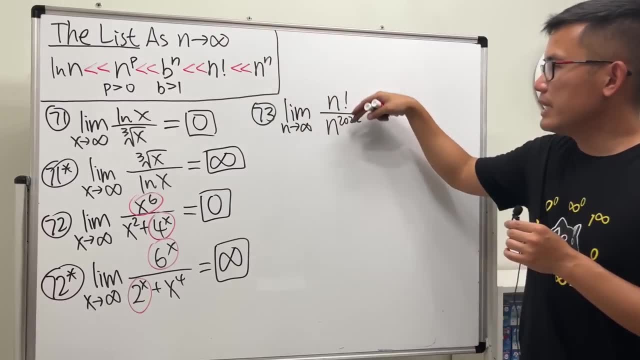 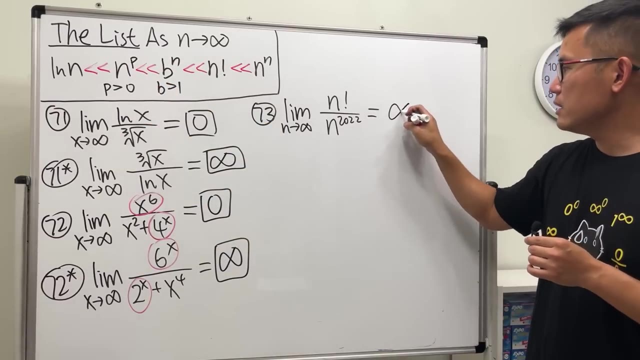 That will be later on, Not now. Anyway, when n goes to infinity, n factorial is so much bigger than n. to the p's power, right This bigger than that. Therefore, the answer is: what Infinity Done? You can give me 1000 of these questions. 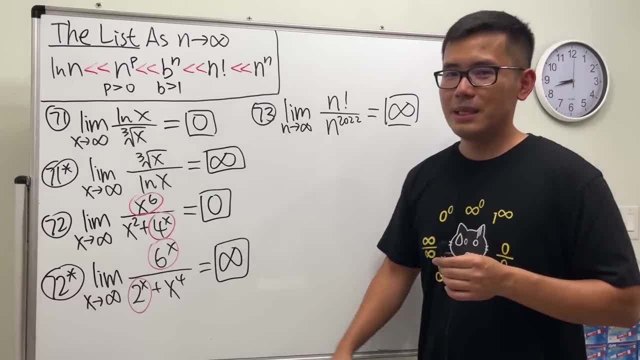 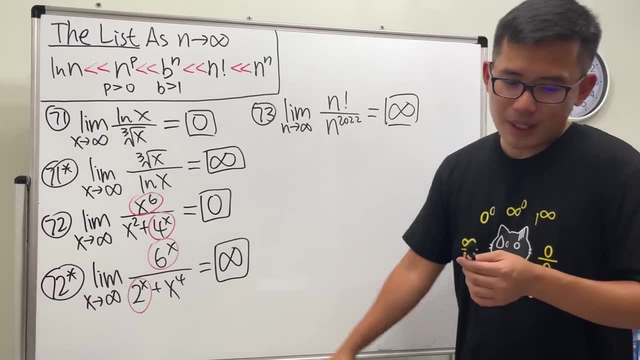 I can finish it. I don't know, I don't want to do it. Actually, you can give me 100 of this question. I can do it in like two hours or one hour, one hour maybe, By the way. 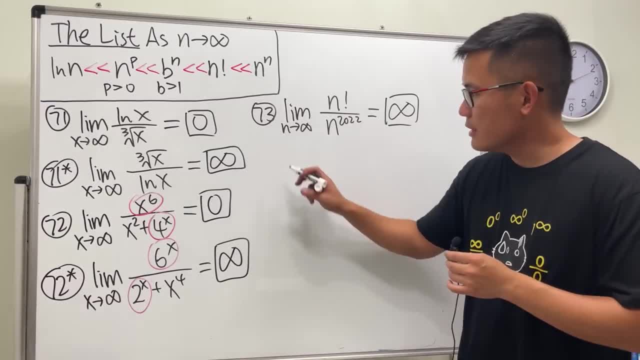 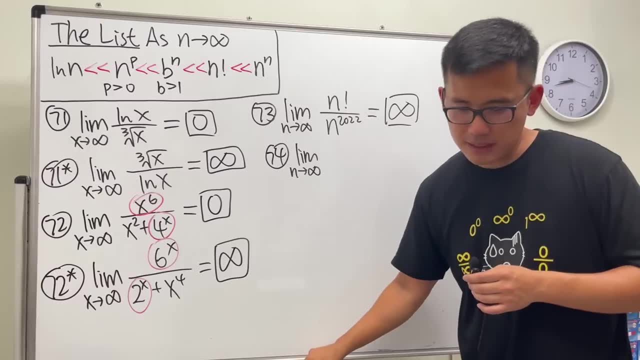 10 seconds, I don't know. Okay, Next 74.. If we have the limit as n goes to infinity. No, I use X Now most of the time we are talking about X. X is much better because we can do L'Hopital's rule. 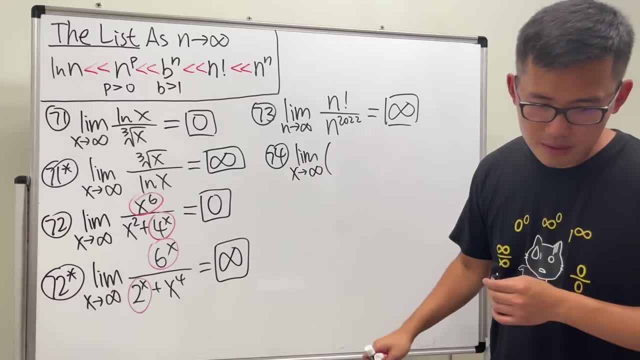 which is like d, dx and all that stuff, But anyway, ln X minus square root of X, Wow. So this is slightly different than these because we have a subtraction here, But just think about the idea. If you have infinity, put it here. 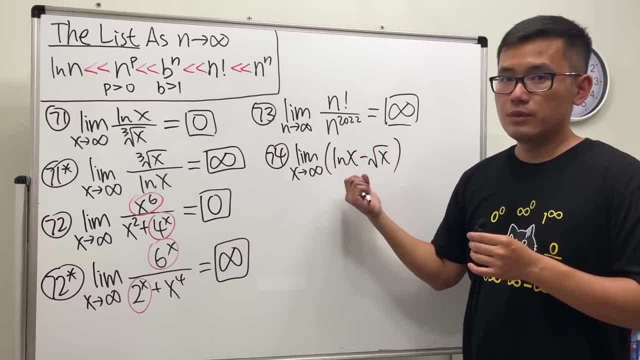 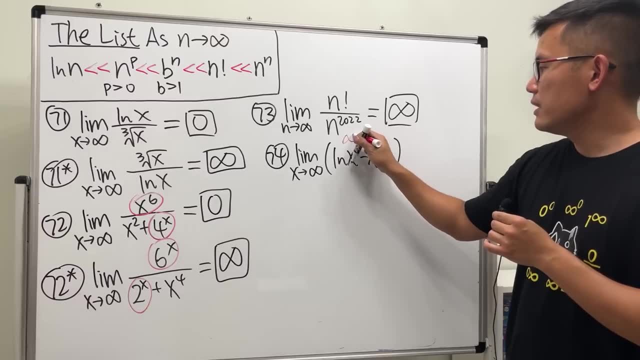 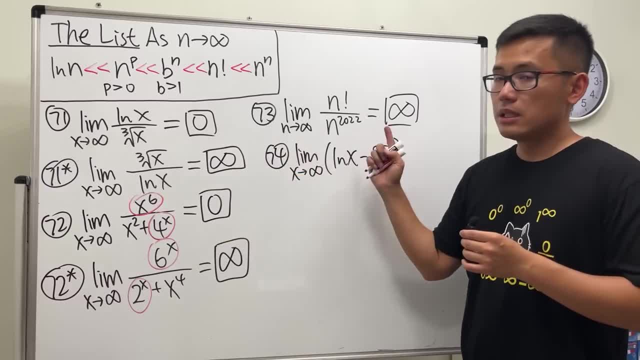 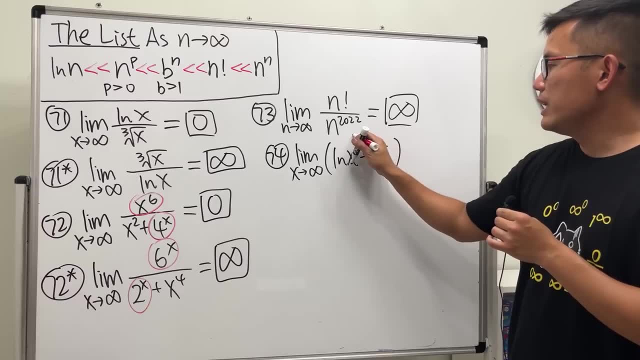 Wow. So this is slightly different than these because we have a subtraction here. But just think about the idea: If you have infinity, put it here, and here we get infinity minus infinity, But one infinity is actually much bigger than the other. 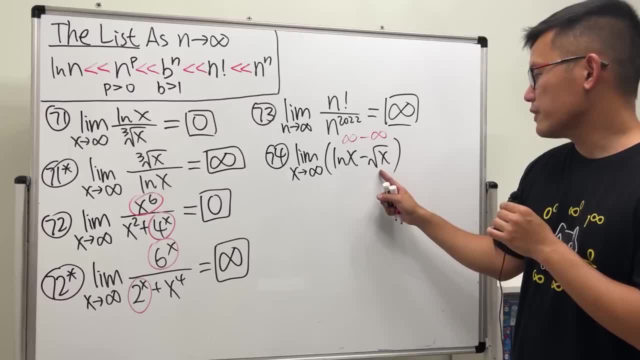 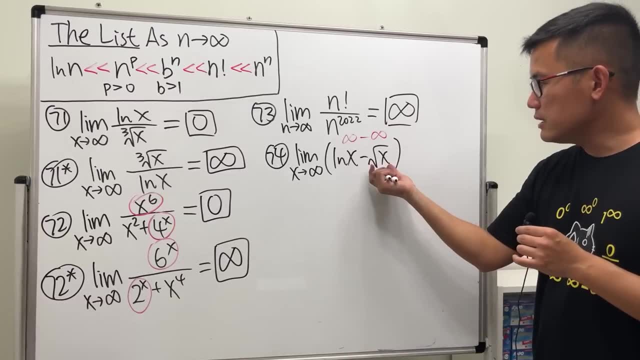 Which one is bigger. This is bigger because square root of x is the same as x to the 1 half power which is here. It's bigger than natural log. So if this is bigger, small minus big, we get negative infinity. 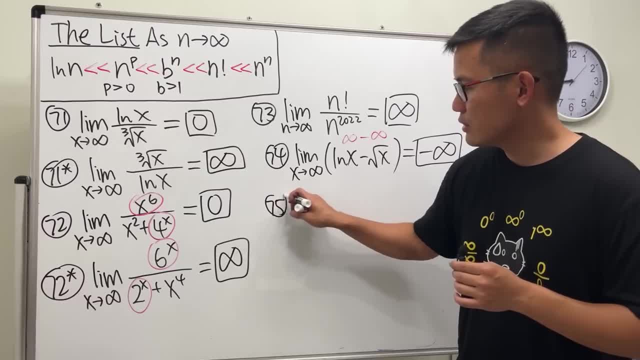 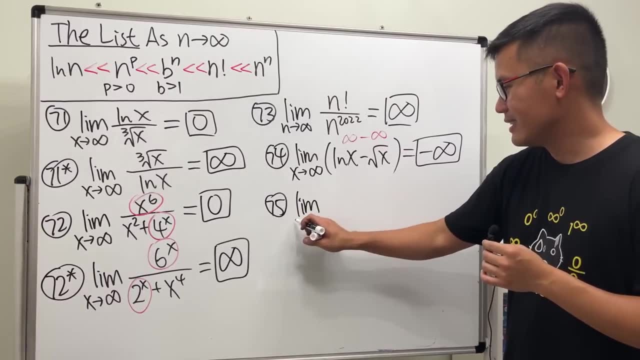 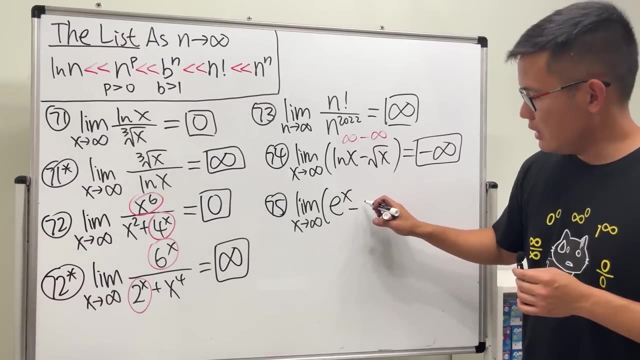 Yeah, just like that. So quick, so fast, so good. Alright, let's try another one. Oh man, this is the one I'm going to miss, Because after this, no more of the list. e to the x minus x to the e. 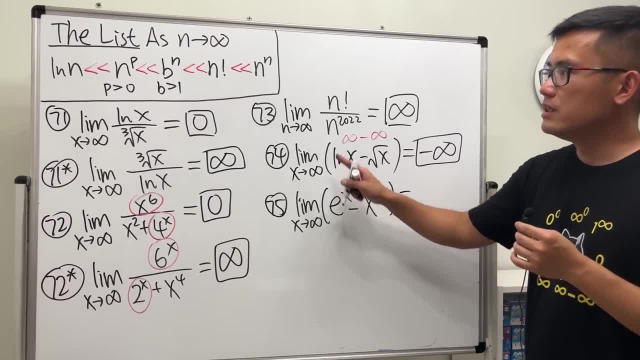 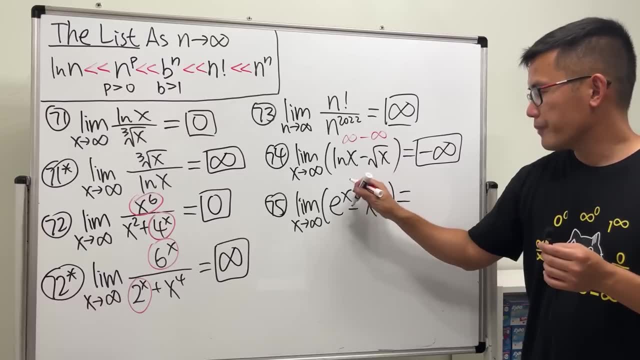 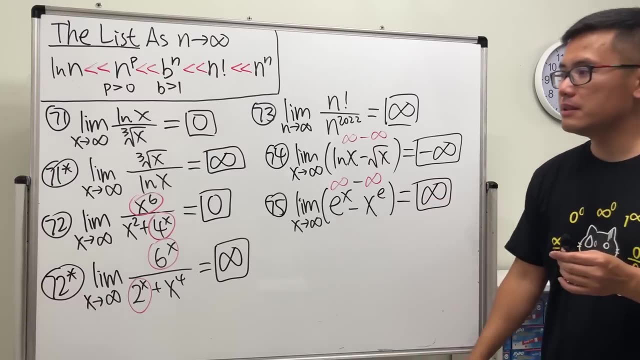 What's the answer? Exponential is much bigger than power. This is x to the power. e right. So this is infinity minus infinity, We get positive infinity. Alright, So you can see, with the list, we can finish a lot of these questions in no time. 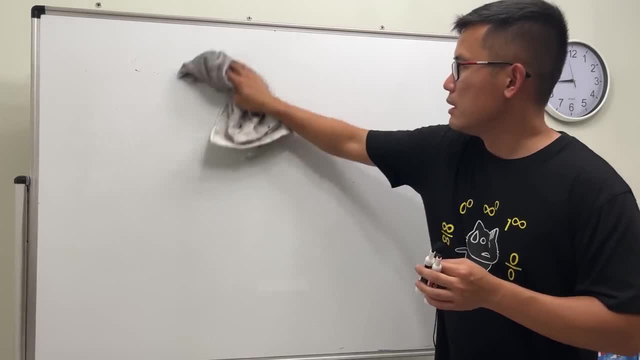 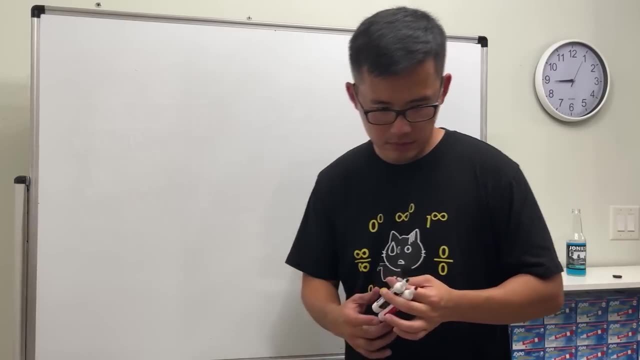 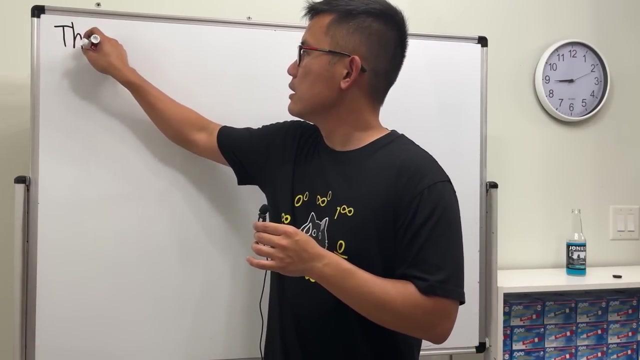 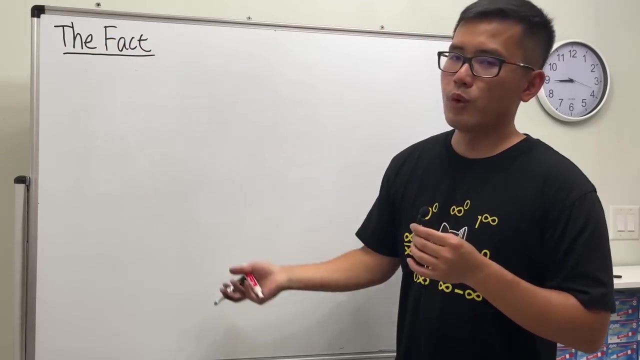 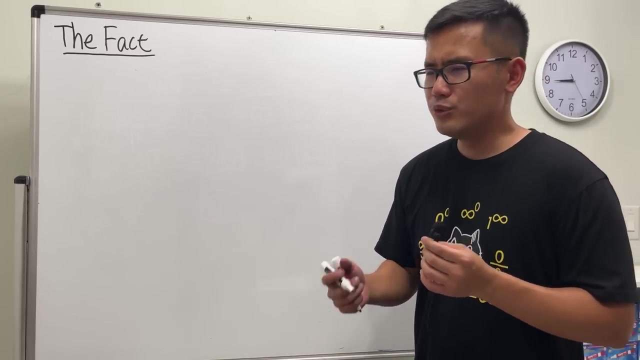 No time applied. Next, I'd like to tell you guys the fact Again. I gave these formulas, these names, Why? Because it's much easier for us to refer them. Yeah, and then, once you have a name with something that you tend to like it more. 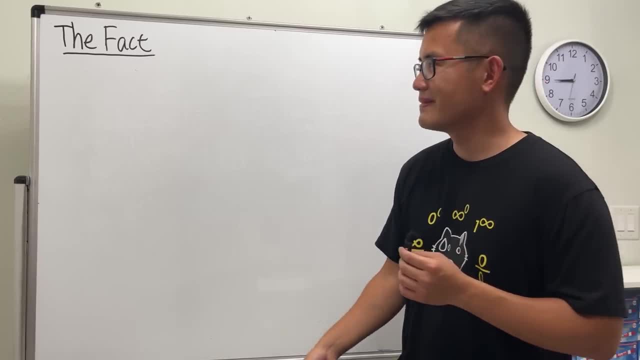 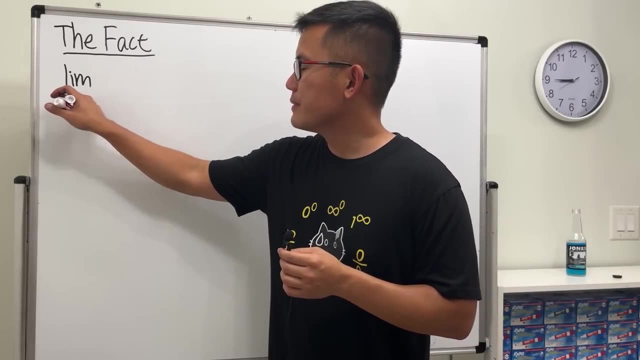 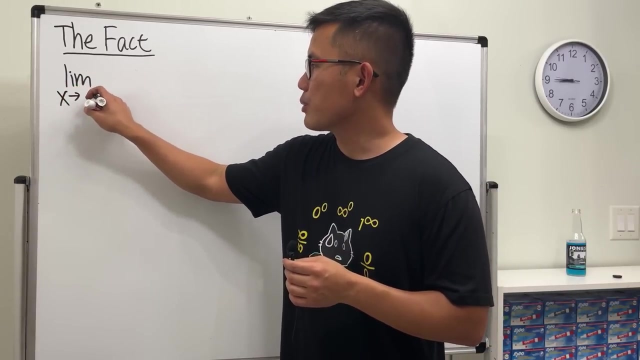 Understanding more and you want to keep it with you more. anyway, The fact I'm just going to write it as the limit and I Don't remember if I use X, what he or what not, doesn't really matter, I'll just use X. X approaching infinity. 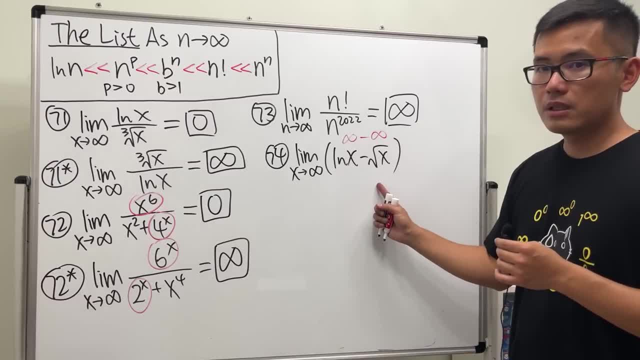 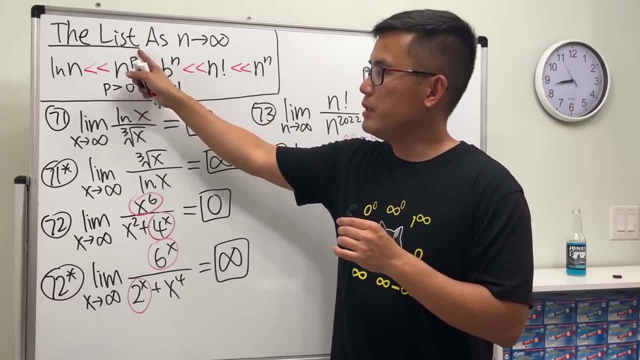 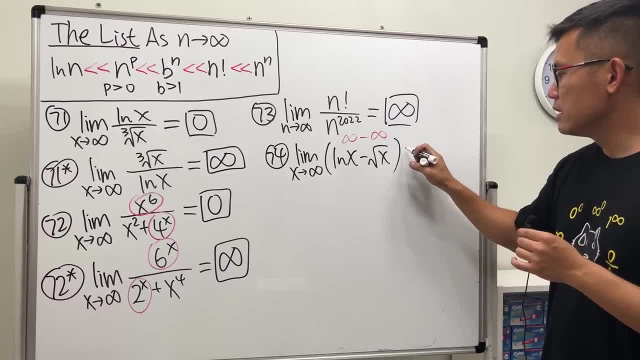 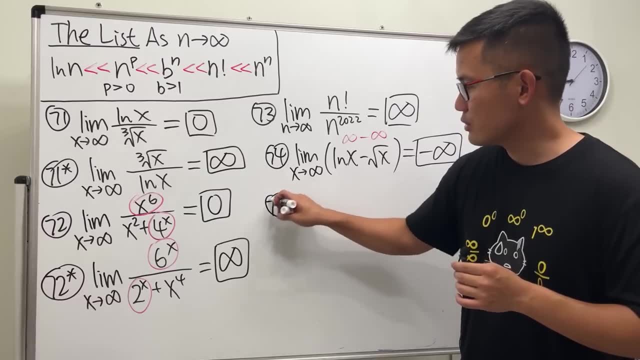 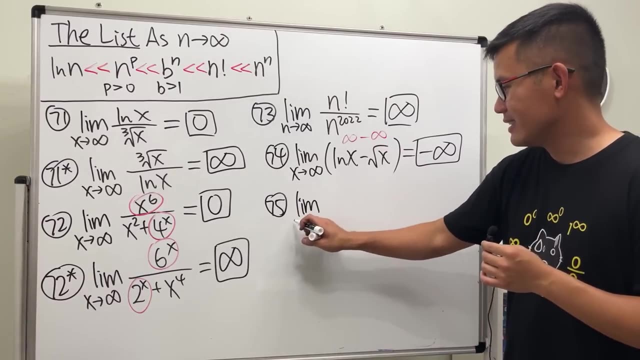 So if this is bigger, small, minus big, we get negative infinity. Yeah, Just like that. So quick, so fast, So good. Alright, let's try another one. Oh man, This is the one I'm going to miss. 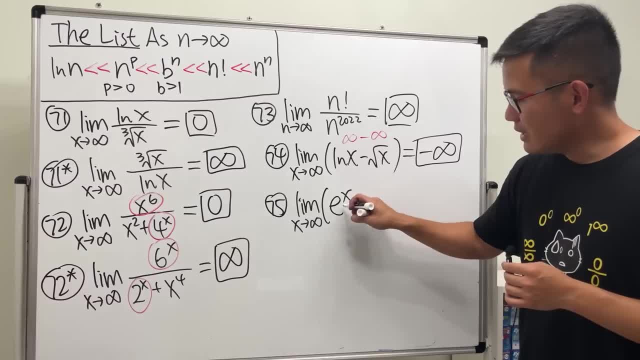 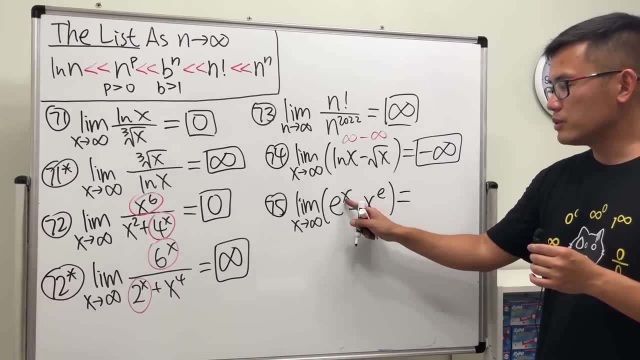 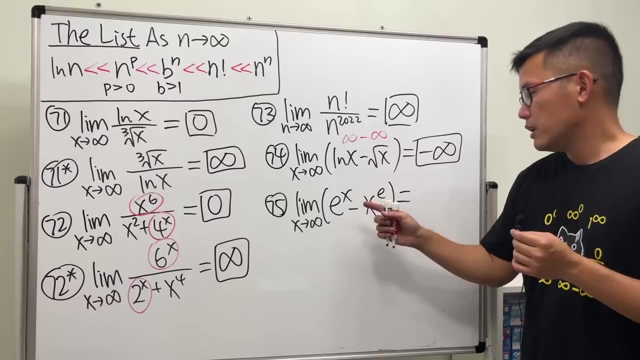 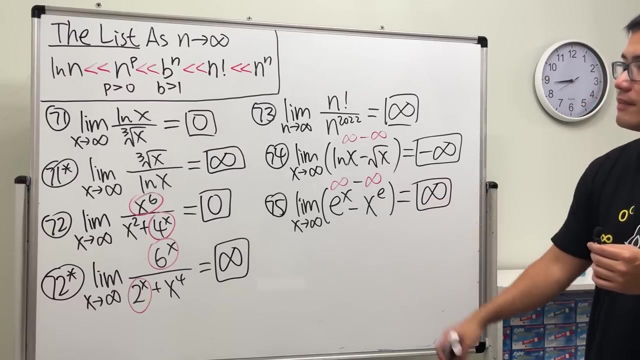 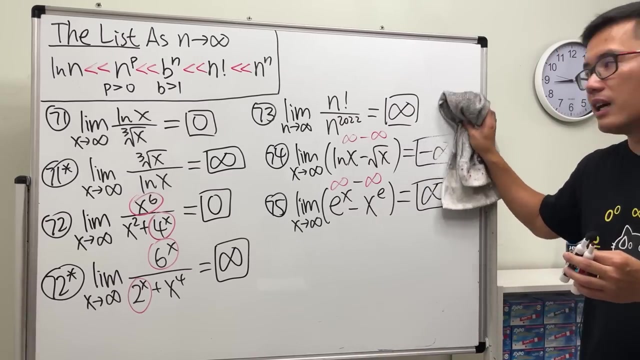 because after this, more the list, e to the x minus x to the e, what's the answer? exponential is much bigger than power. this is x to the power, e, right. so this is infinity minus infinity, we get positive infinity. all right, so you can see, with the list we can finish a lot of these questions in no time. 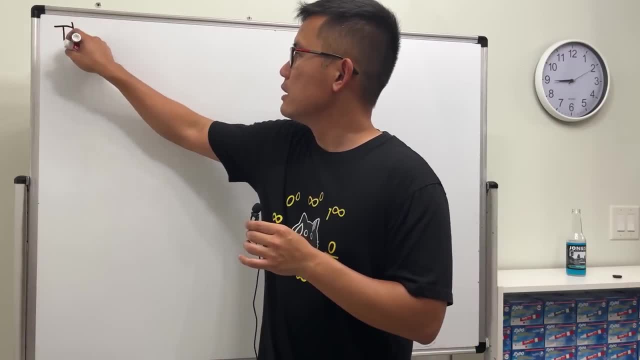 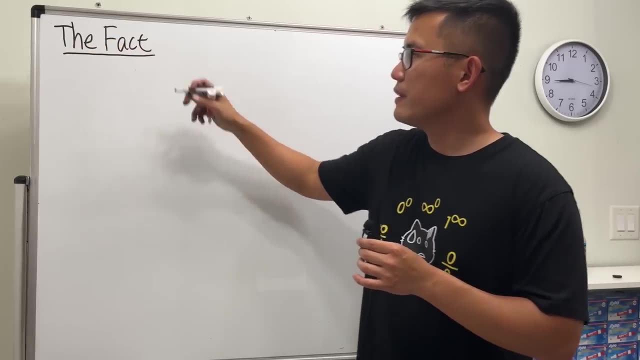 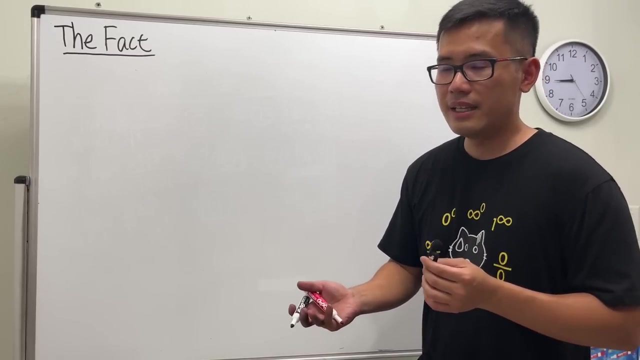 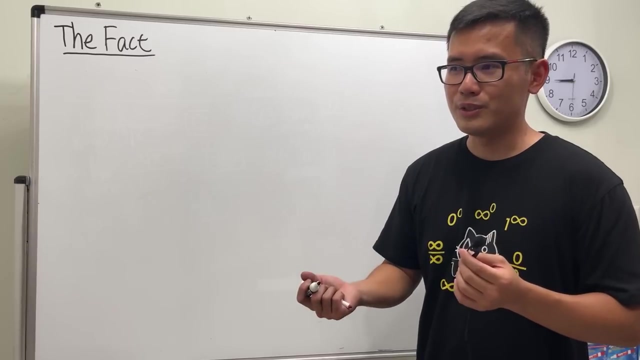 next, i would like to tell you guys the fact again. i gave this formula, these names, why? because it's much easier for us to refer them. yeah, and then, once you have a name with something that you tend to like it more, understand it more and you want to keep it with you more anyway, 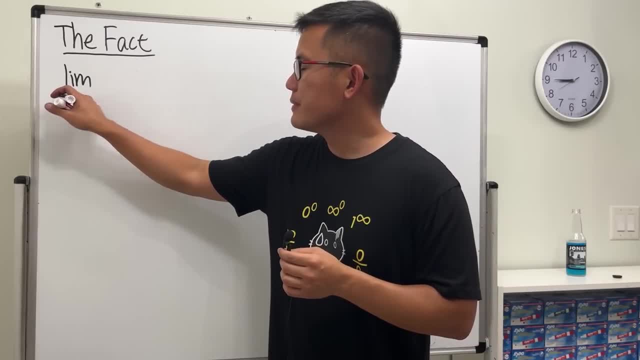 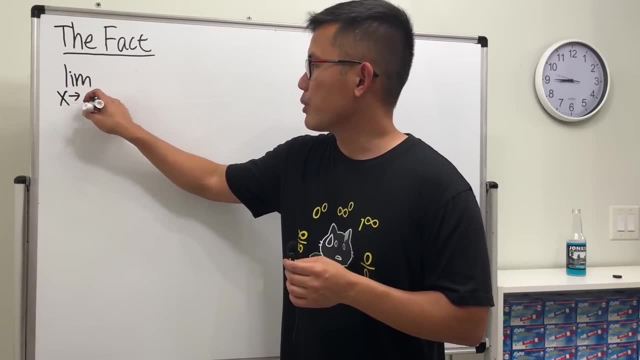 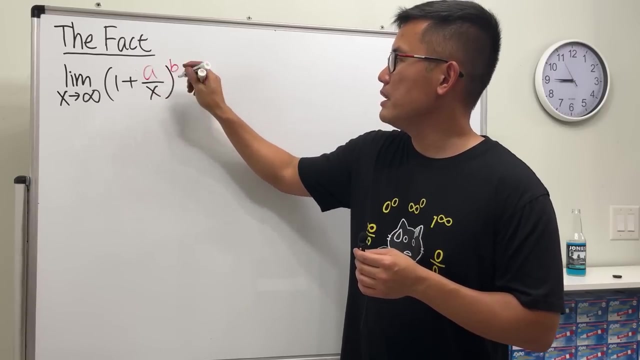 the fact. i'm just going to write it as the limit and i don't if i use x. what he or what not doesn't really matter. i'll just use x, x approaching infinity, if you have one plus some number: a over x, raised to the b, x power. 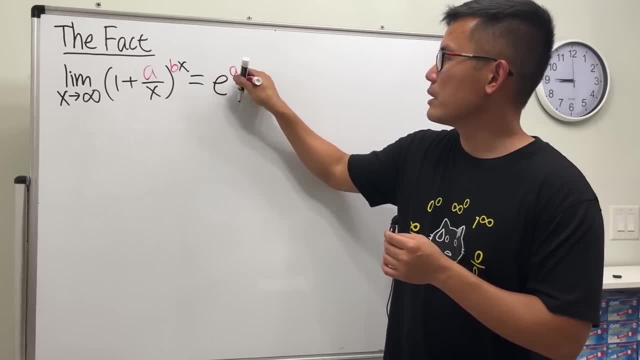 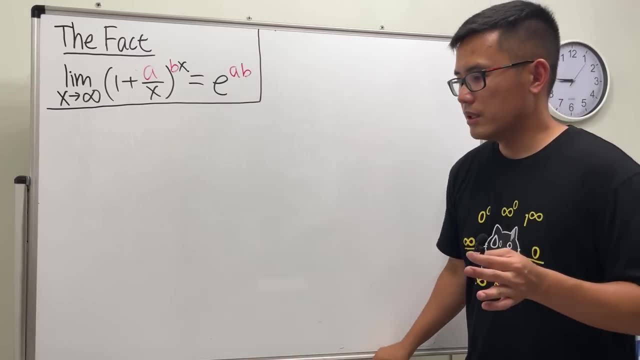 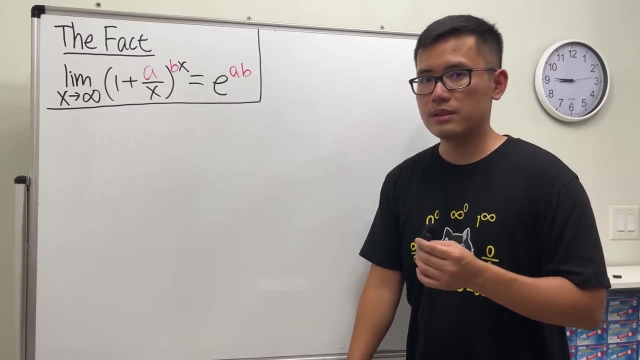 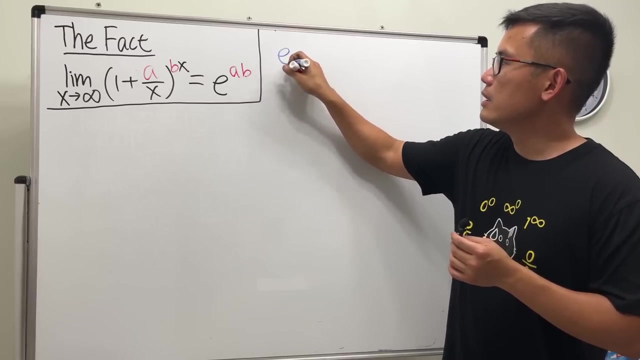 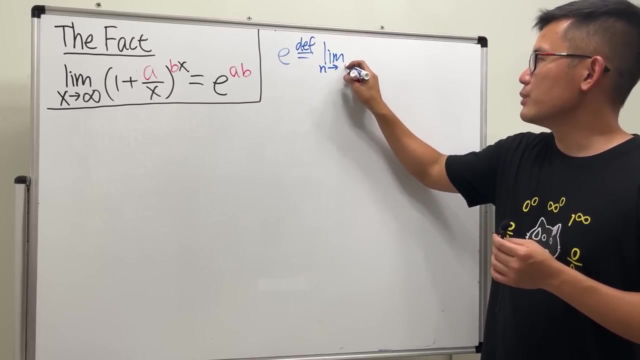 this right here gives us e to the a b power. this is it. and this right here is actually nothing, nothing special. you actually have seen it before. you just never recognize it, uh, from your pre-calculus class with that calculus questions that you have been doing. so here's the deal. we define e to be the limit as n x. one knot doesn't really matter seriously. 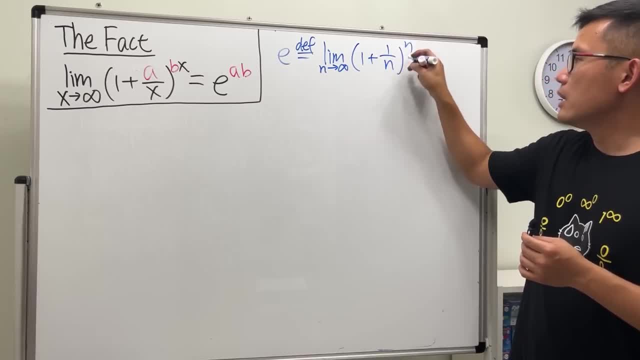 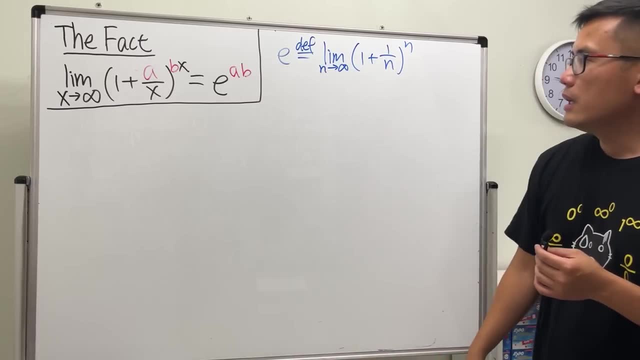 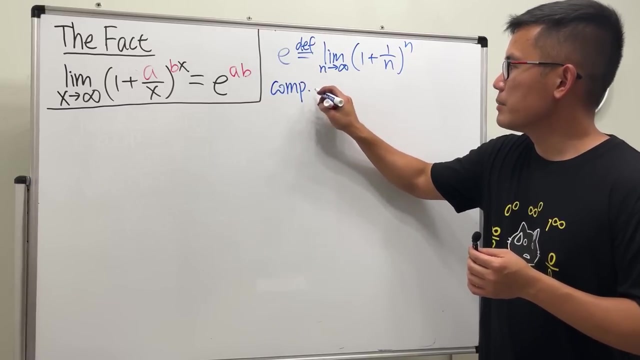 and let me use n, and this is just one of the definitions, so you can take this for the definition of the number e, which is about 2.7 each. all right, all right, and if you guys recall your compound interest formula, so this is the compound. 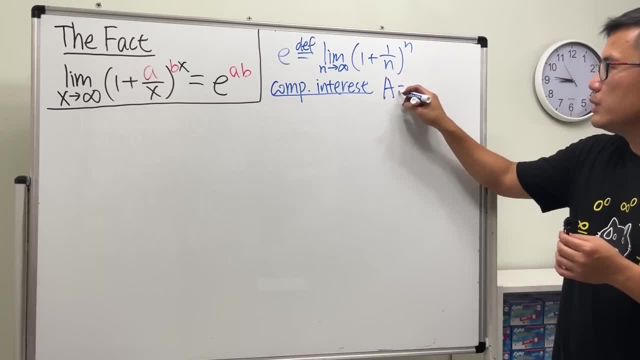 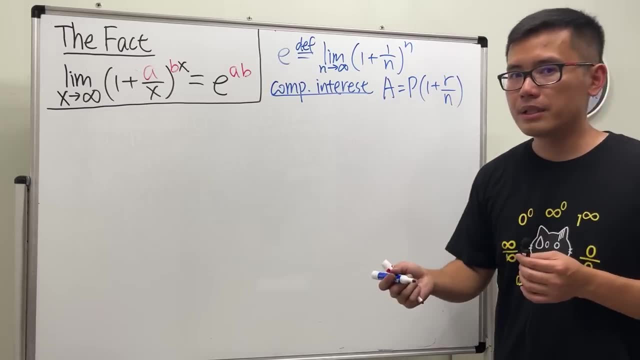 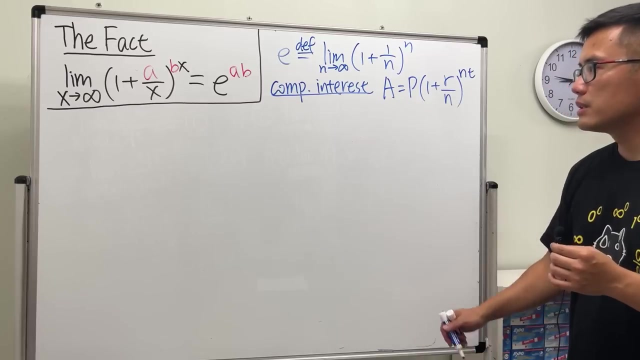 interest formula. you have the amount. it's equal to the principle times one plus r, which is the interest rate divided by however many times you count on a year, and then raised to the n t's power. t is the number of years. so this is the compound interest formula. i will have to say that. 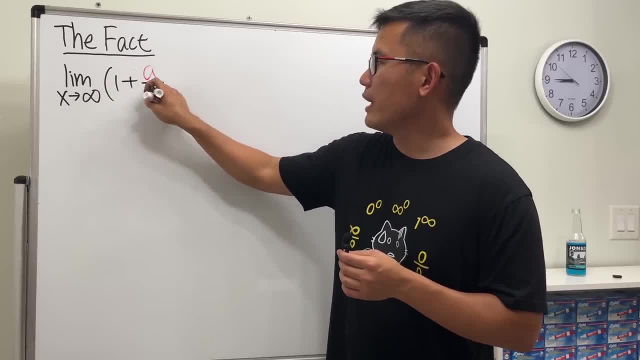 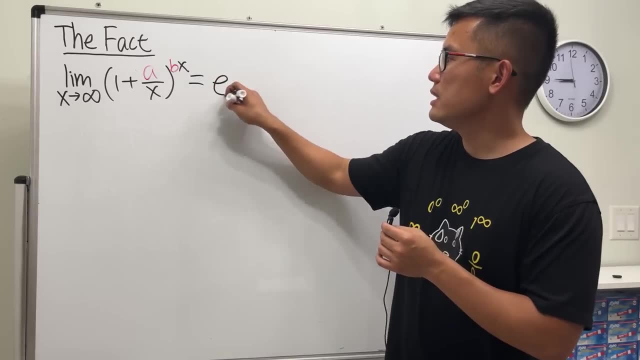 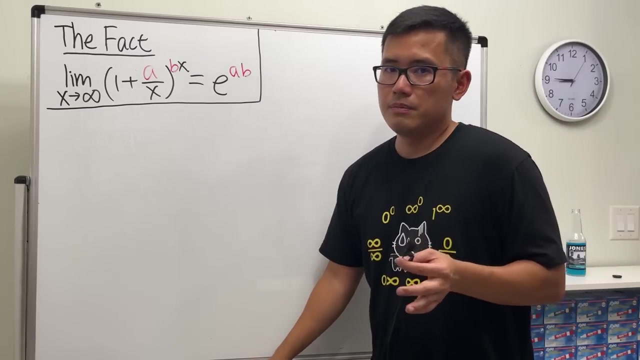 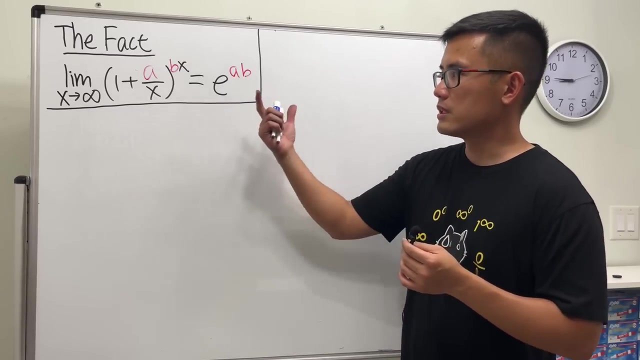 If you have one plus some number a over X raised to the B X power, This right here gives us e to the a B power. This is it, And this right here is actually nothing, nothing special. You actually have seen it before. it just never recognized it From your precalculus class with like a calculus questions that you have been doing. So here's the deal. 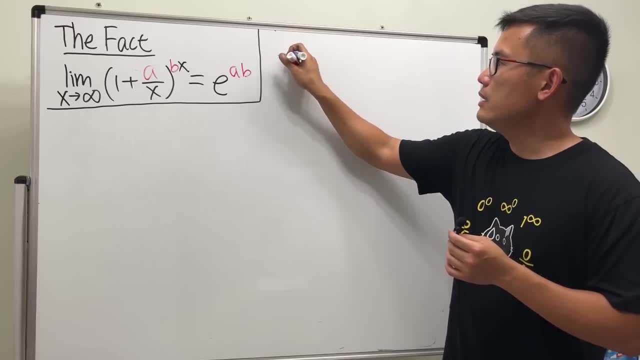 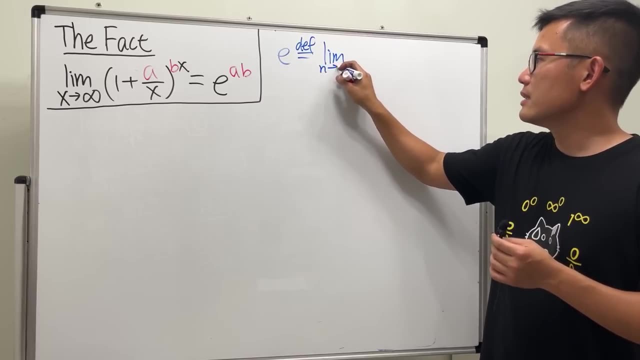 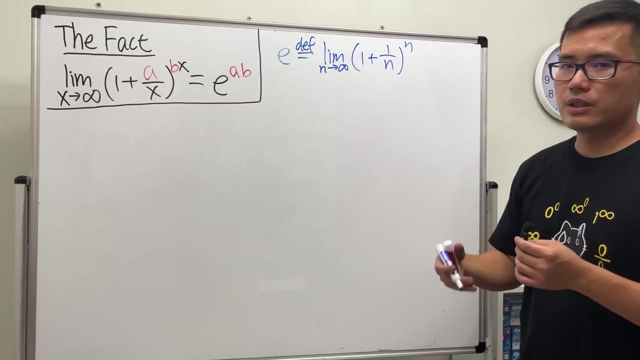 We defined E to be The limit as n X, 1, not doesn't really matter seriously, and let me use n, And this is just one of the definitions, so you can take this for the definition of the number e, which is about 2.7 each. all right, and 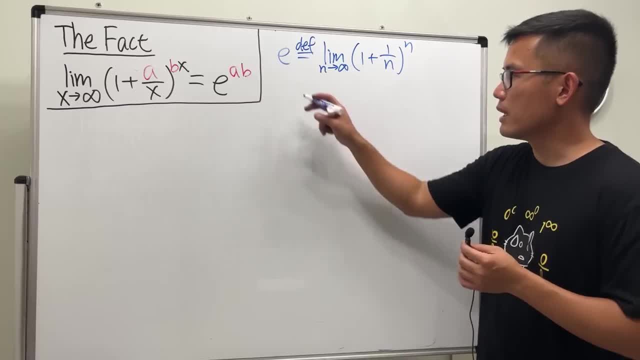 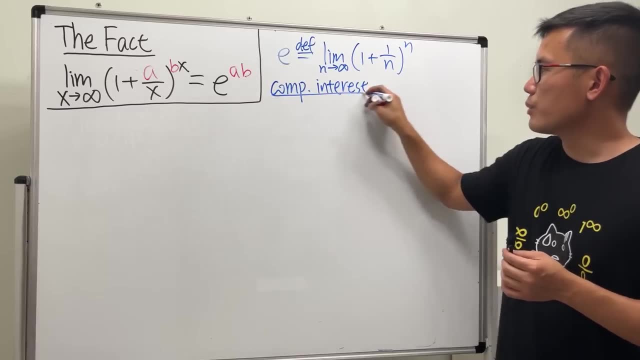 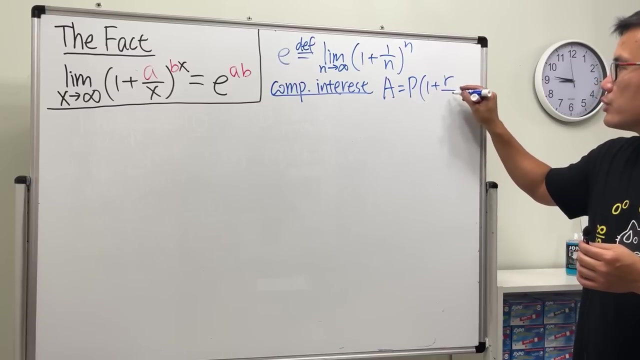 if you guys recall your compound interest formula. so this is the compound interest formula, Interest formula. You have the amount it's equal to the principal times 1 plus R, which is the interest rate divided by however many times you come from a year, and then raised to the n. 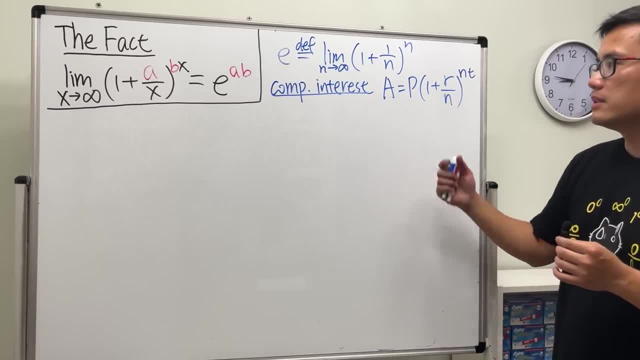 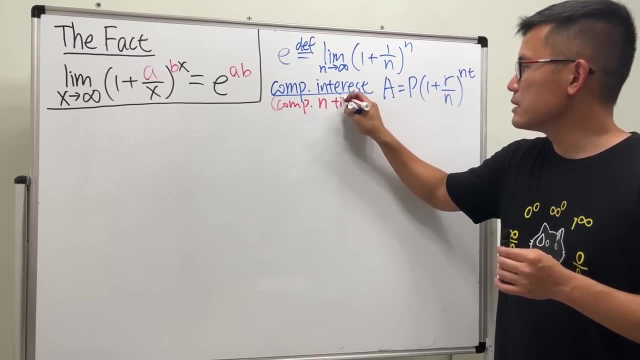 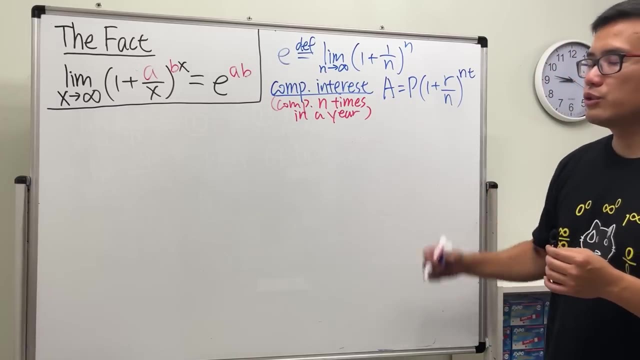 T's power. T is the number of years. So this is the compound interest formula. I will have to say that Compound n times In a year So you can see a difference in the amount of interest rate that you earn every day. Right? so that should be clear and you guys should have seen this back in precalc. 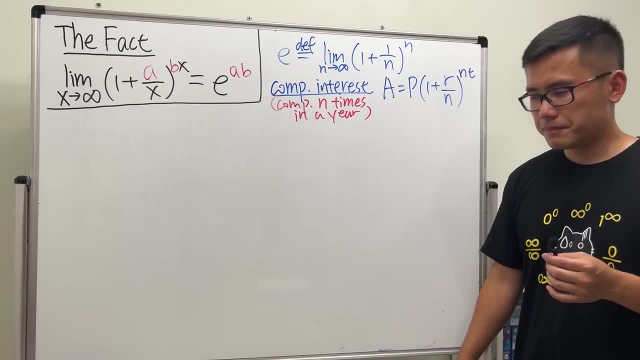 well, if you just continues, if you- Let me give you an example- If you put money that say $1,000, into the bank that will give you interest, right, Then the way that they do it- I believe most of them do it- is they will compound every day. 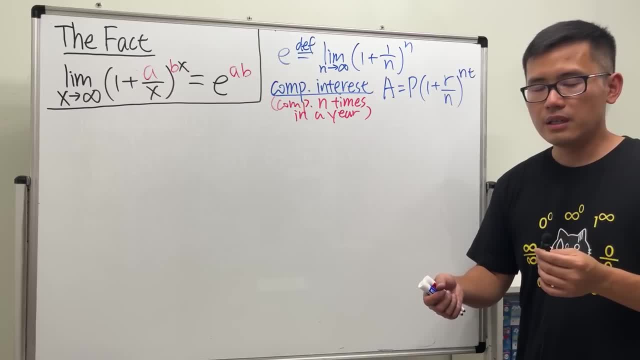 So they will compute the interest that you earn every day, Okay, but they will pay you every month. So the idea is that if you have $1,000 in this bank, which is like $1,000 per month, right? So the idea is that if you have $1,000 in this bank, which is like $1,000 per month, right? 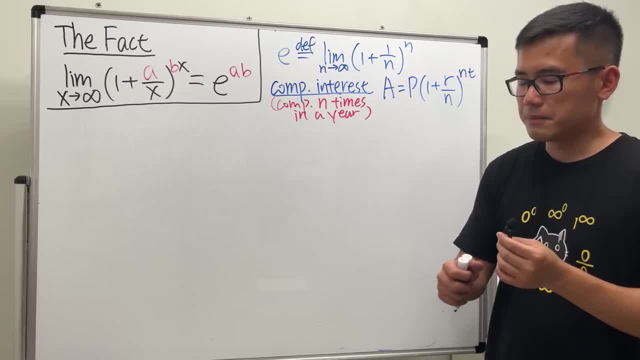 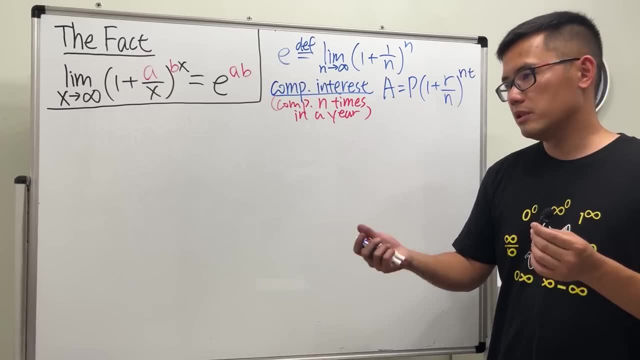 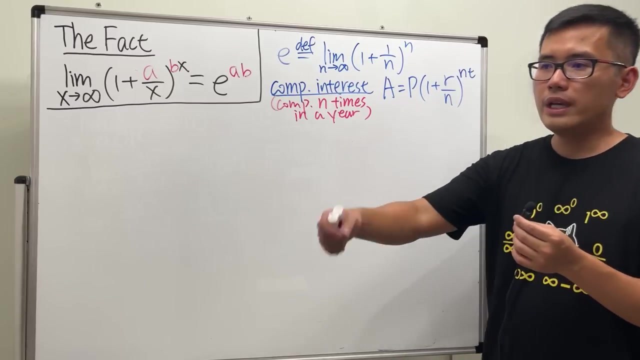 there. if you have- i'm saying regular banking, if you want to withdraw tomorrow, guess what? you will still have one thousand dollar. if you withdraw in two days, you still have one thousand dollars. okay, that regular checking account will saving account. you have to wait until a month later. 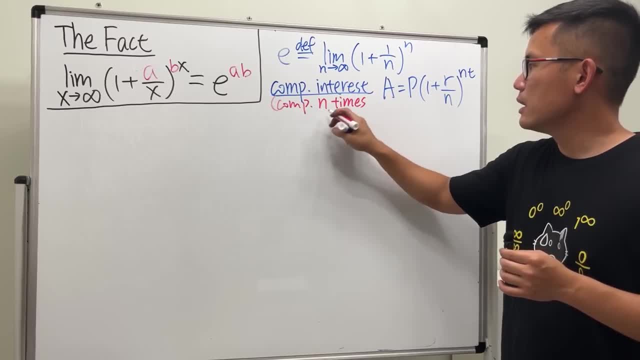 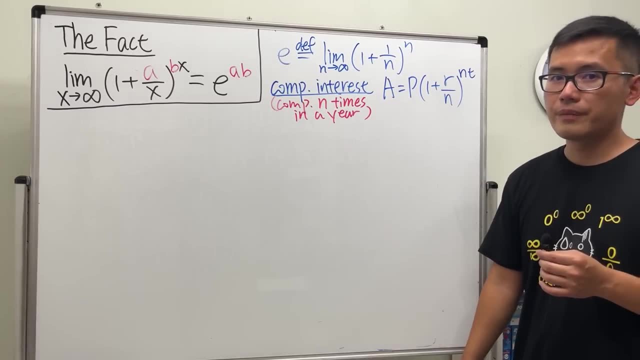 compound n times in a year, right. so that should be clear and you guys should have seen this back in pre-calc. well, if you just continues, if you let me give you an example: if you put money, let's say one thousand dollars- into the bank will give you interest, right. then the way that they do it- i believe most of them do it- is they. 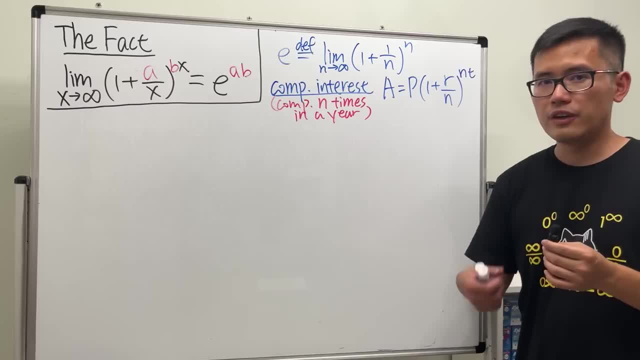 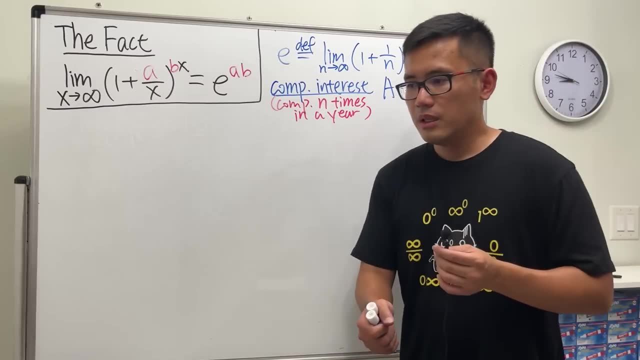 will compound every day. so they will compute the interest that you earn every day, okay, but they will pay you every month. so the idea is that if you have one thousand dollar in there, if you have, i'm saying, regular banking, if you want to withdraw tomorrow- guess what, you will still have one. 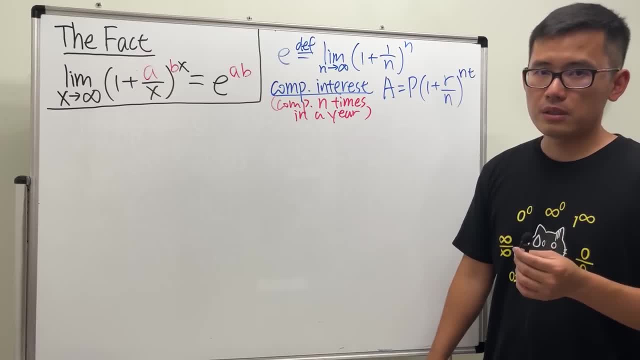 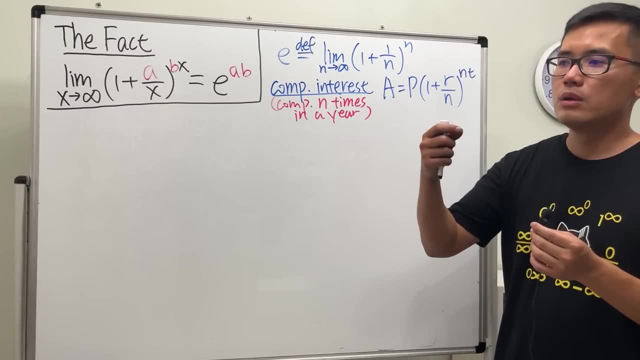 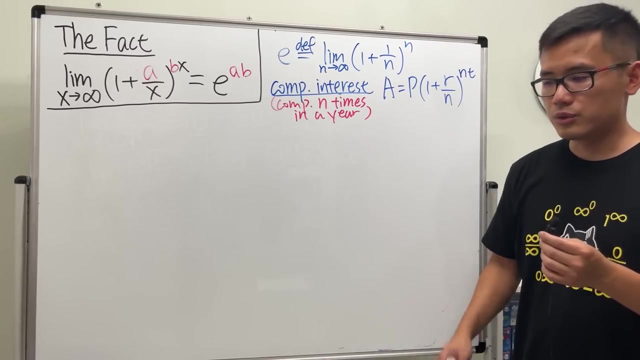 thousand dollar. if you withdraw in two days, you still have one thousand dollars. okay, that regular checking account or saving account. you have to wait until a month later and they will just kind of just keep track of all the interest that you have earned throughout the months and then you get paid per month, that's. 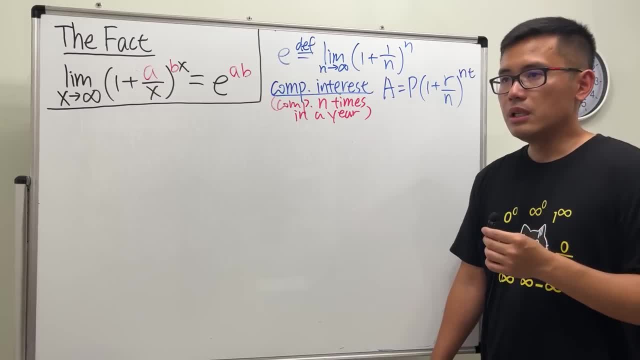 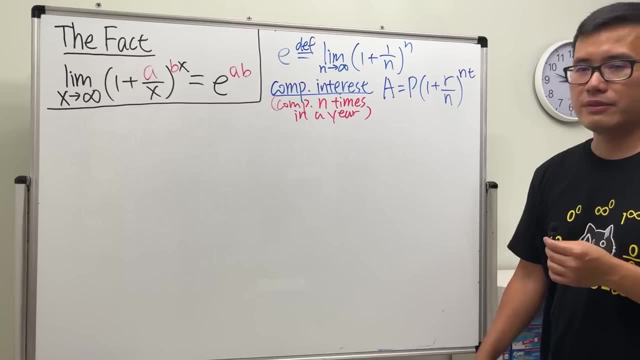 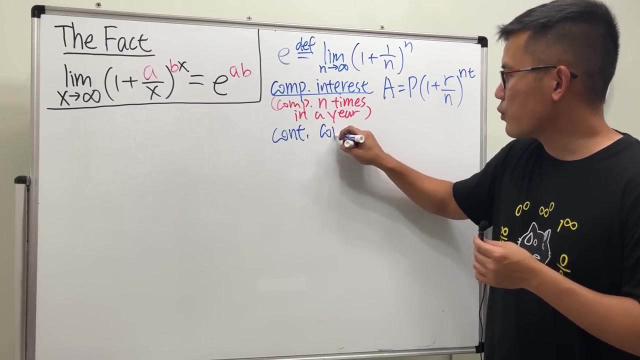 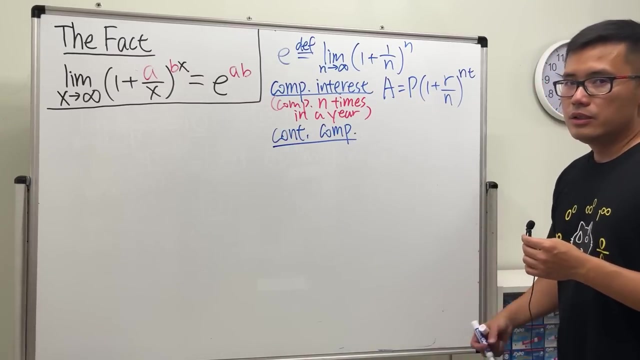 pretty much how it works. anyway, imagine if you can get continuous compound. well, in real life that's not possible, but in math the idea is just: you take the limits and goes to infinity, so you have the continuous compounds for formula- all right. and continuous common formula is like a continuous growth, and that's how you can get the exponential. 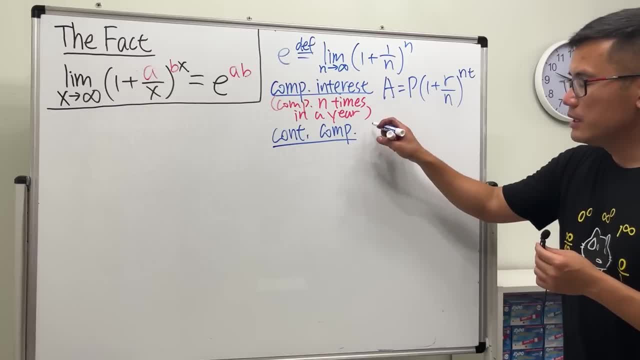 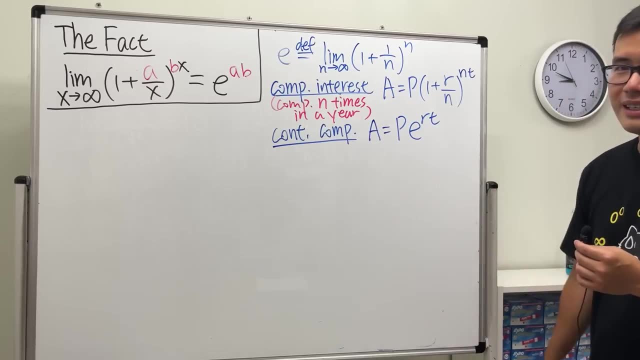 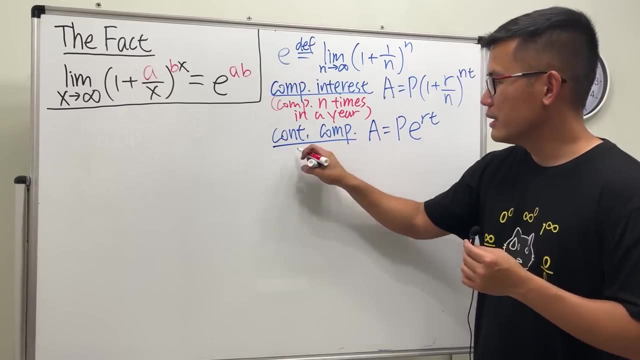 growth or decay depends on how you look at it. but you will see, this is the famous pert formula: amount is equal to p? e r t pert formula. where's the e? well, e is precisely because we are talking about continuous. that means n goes to infinity. you pretty much compound infinitely many times in a year. 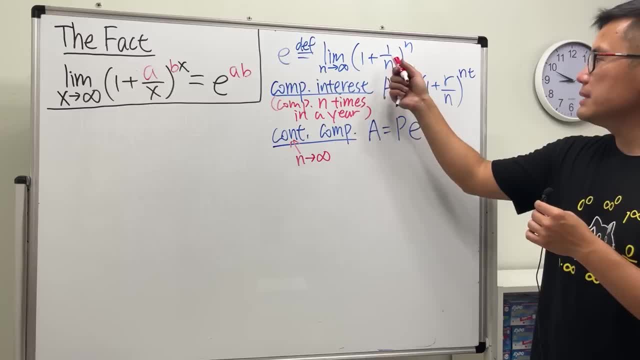 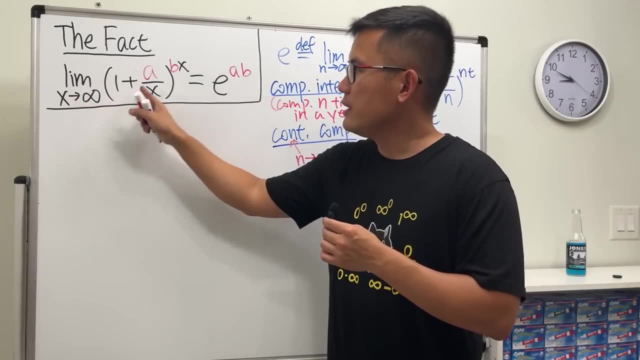 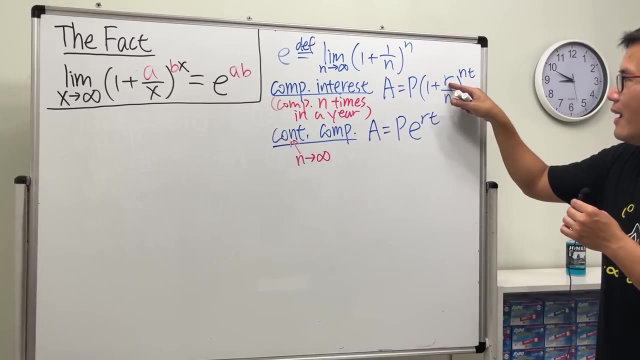 and you see, precisely is this: as n goes to infinity, this part gives you the e. so we have the e, and you see it right here. as x goes to infinity, this and that is the exponent of e. just like this, the so-called continuous compound formula r, t is the power of e, right here, and this is just like a. 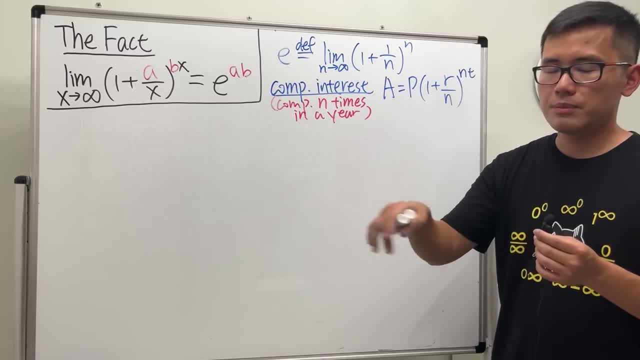 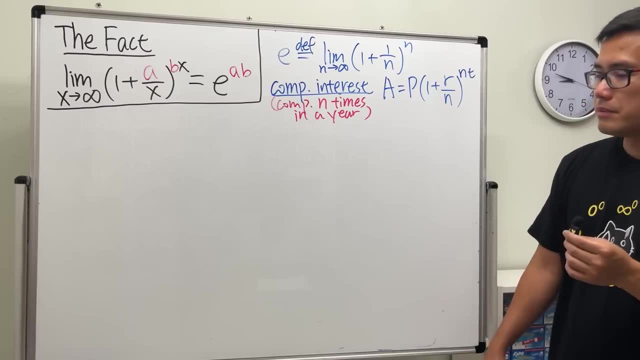 and they will just kind of just keep track of all the interest that you have earned throughout the months, and then you get paid per month. that's pretty much how it works anyway. imagine if you can get continuous compound. well, in real life that's not possible, but in math. 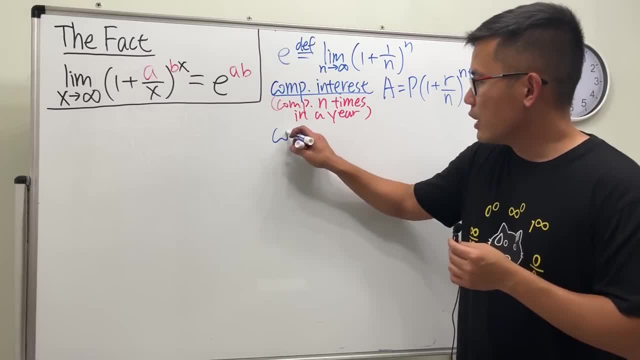 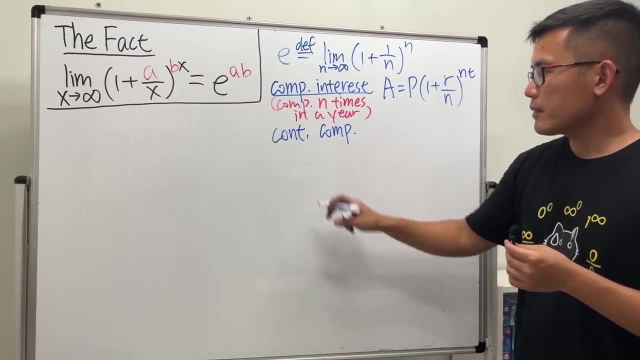 the idea is just you take the minutes and goes to infinity, so you have the continuous compound formula- all right, and continues comfort formulas like a continuous growth, and that's how you can close it down. this is all how you can close it down so you can stop all these things could be. 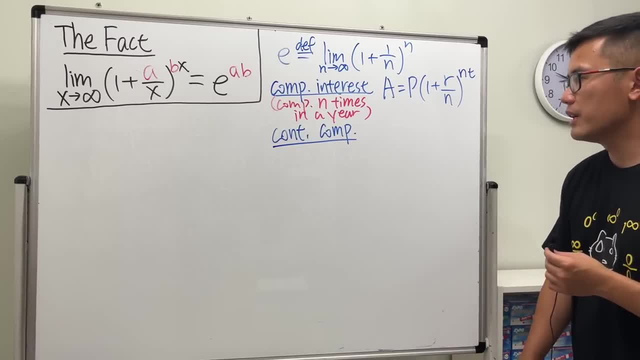 large, you can move sophisticatedtake a continuous growth, and that's how you can get the exponential growth or decay, depends on how you look at it. but you will see, this is the famous pert formula: amount is equal to p? e r t pert formula. where's the e? well, e is precisely. 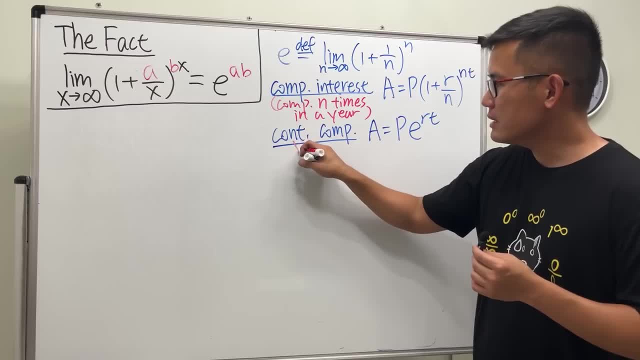 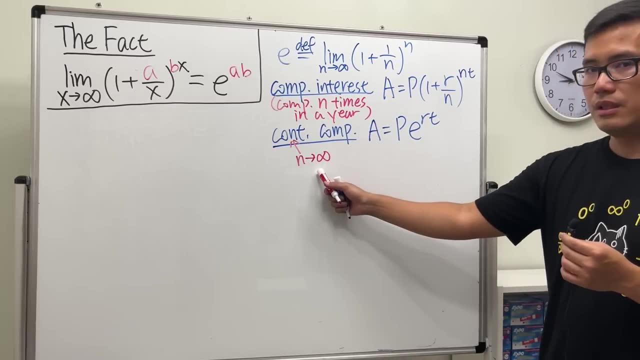 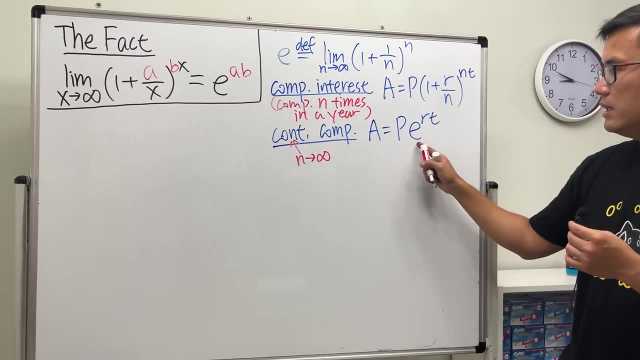 because we are talking about continuous. that means n goes to infinity. you pretty much compound infinitely many times in a year and you see, precisely is this: as n goes to infinity, this part gives you the e, so we have the e, and you see it right here. as x goes to infinity, this and that. 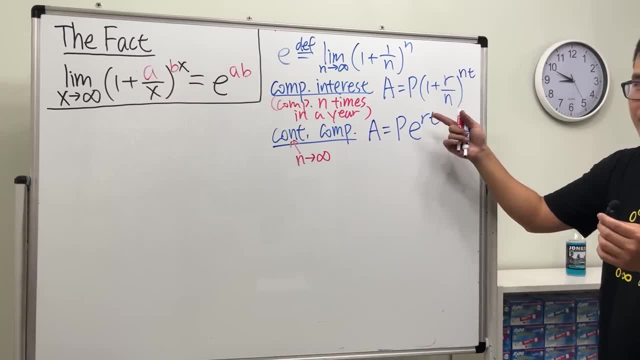 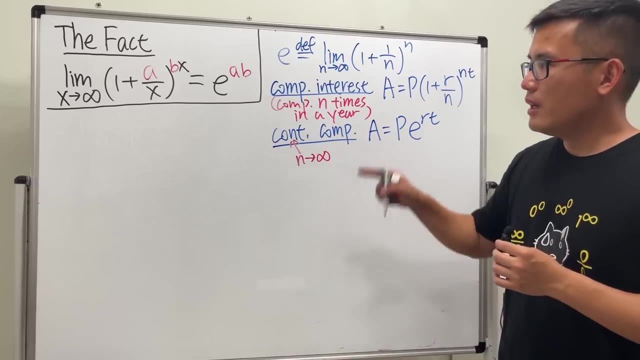 is the exponent of e, just like this. so the so-called continuous compound formula r, t is the power of e right here, and this is just like a coefficient. so you actually have seen this before. yeah, anyway, remember this formula, then you can use it and i'll show you guys how. 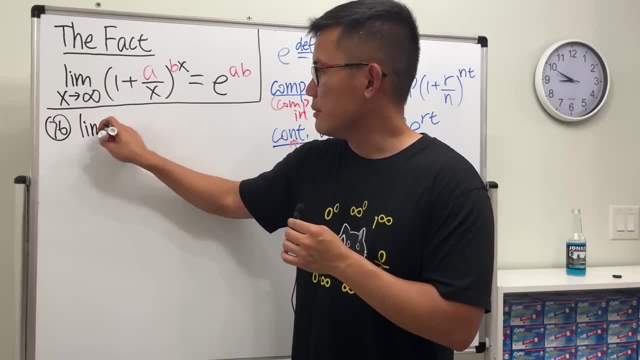 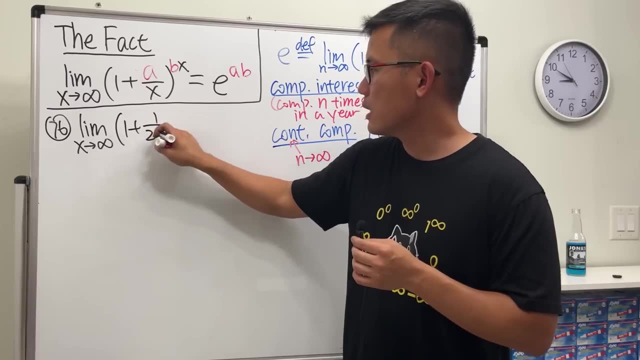 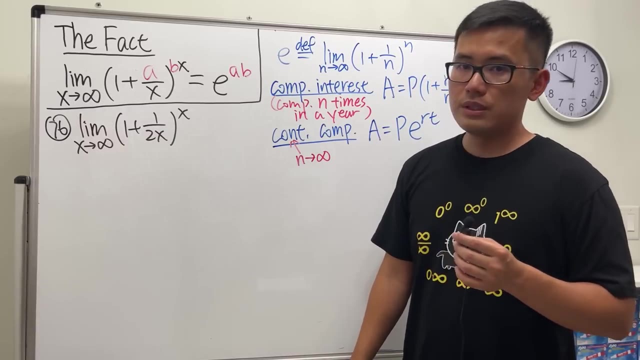 number 76. take a look at the limit as x approaching infinity, and we have 1 plus 1 over 2x raised to the x power. cool, all right, i tell my students you do this, identify the a and b, and then pretty much use it. what's the a, though? 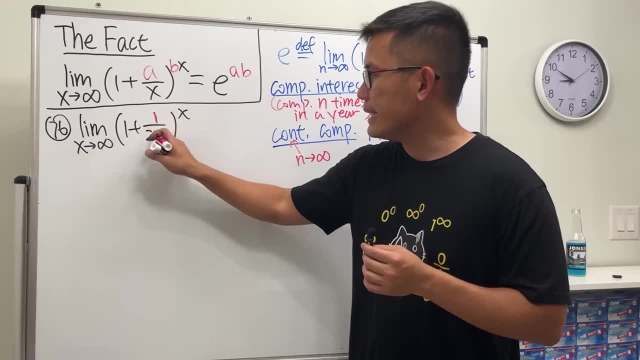 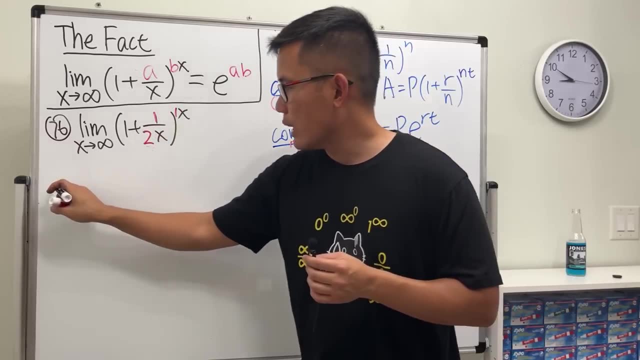 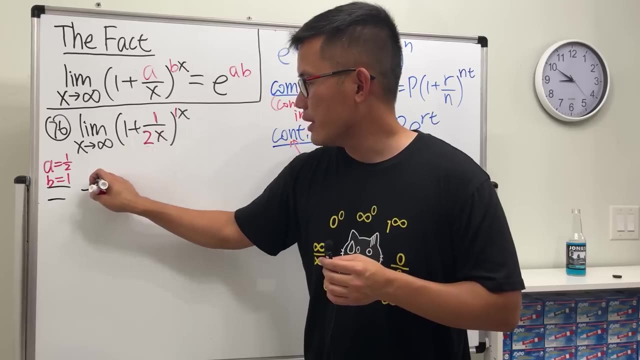 pay attention: right here is that a is actually 1 over 2. right, it's 1 over 2 and then b is 1. so i would write it right here: a is 1 over 2 and b is equal to 1. so this right here is just e to the 1 over 2 times. 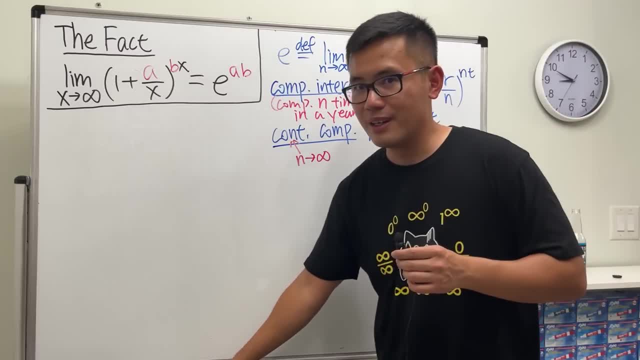 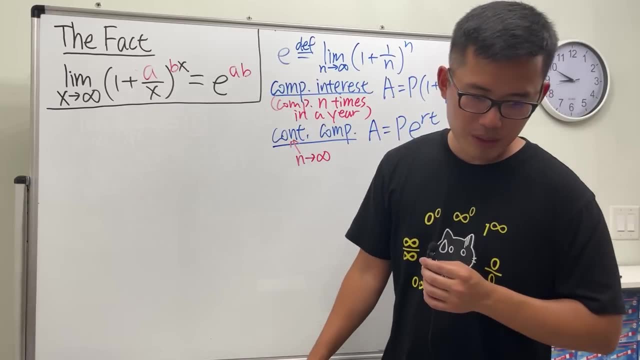 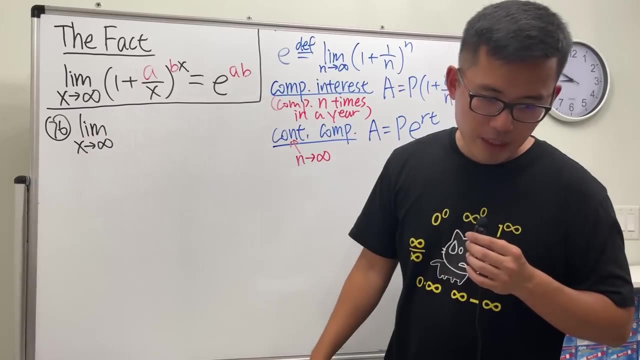 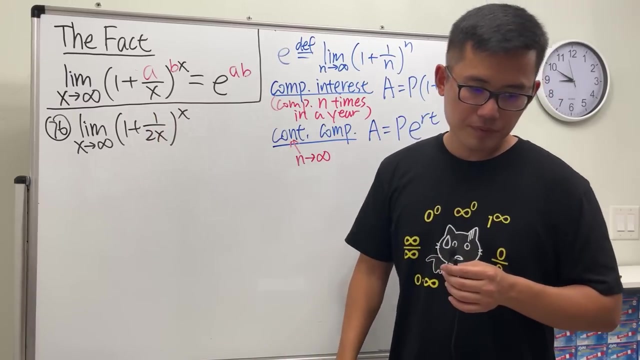 coefficient. so you actually have seen this before. yeah, anyway, remember this formula, then you can use it and i'll show you guys how. number 76- take a look at the limit as x approaching infinity and we have 1 plus 1 over 2x raised to the x power. cool, all right, i tell my students you do this. identify the a and b. 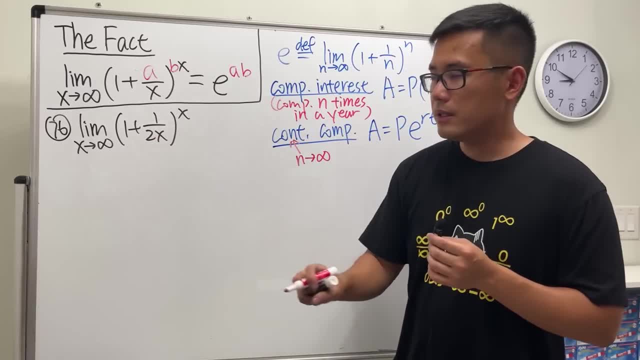 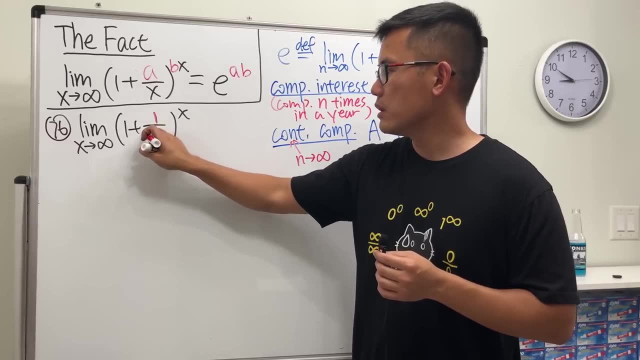 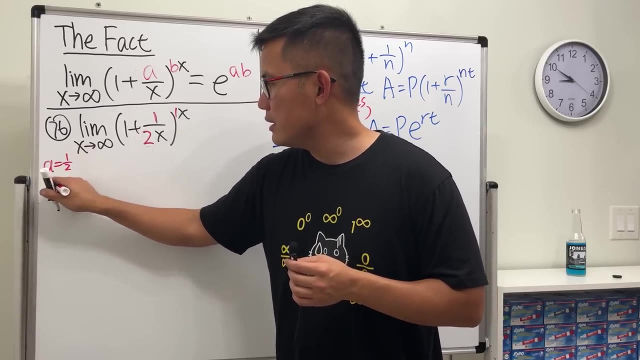 and then pretty much use it. what's the a, though? pay attention, right here is that a is actually 1 over 2. right, it's 1 over 2 and then b is 1, so i would write it right here: a is 1 over 2 and b is. 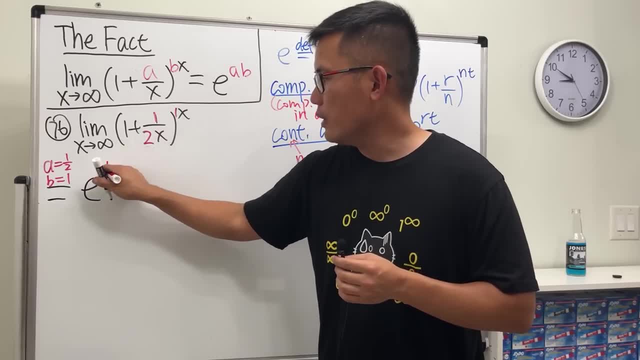 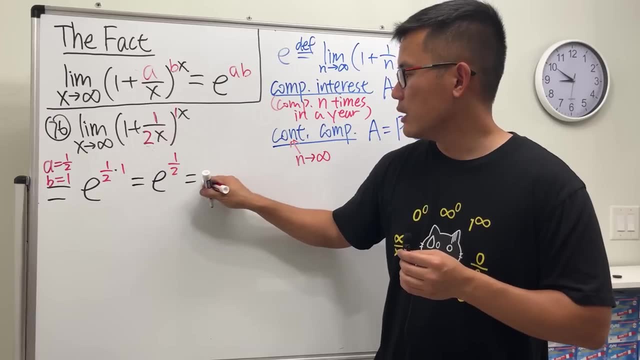 equal to 1. so this, right here, is just e to the 1 over 2 times 1, which is just e to the 1 over 2 power, which is just the square root of e to the 1 over 2 power, which is just the square root of. 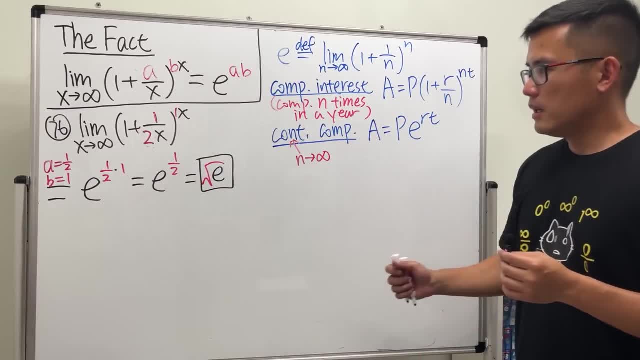 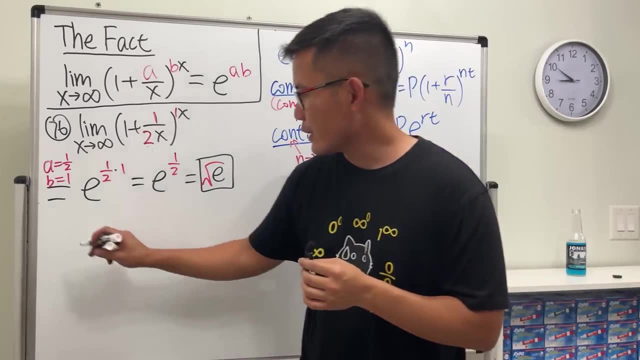 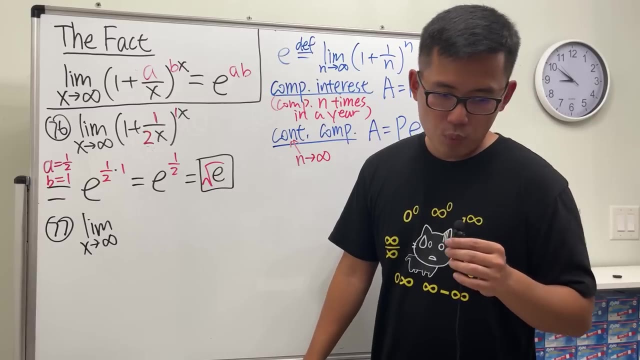 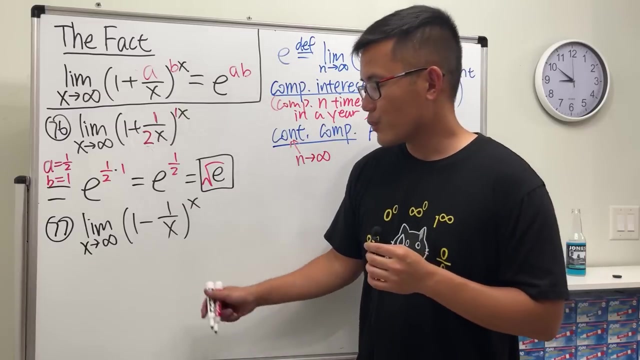 e all right, okay, so that's the answer for that, nice and quick. now try another one: 77 limit as x approaching infinity, and then we have one plus one, minus this to the x power. so what's the a value, the i here, negative one. good, yeah. 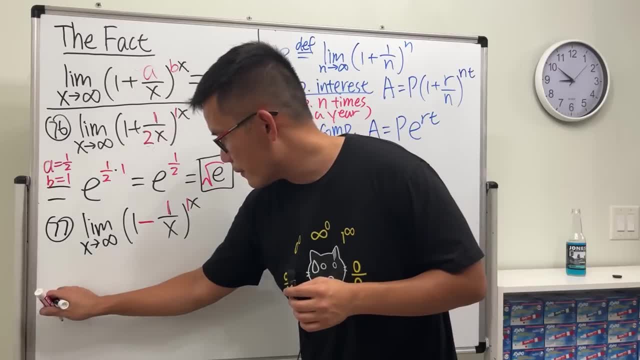 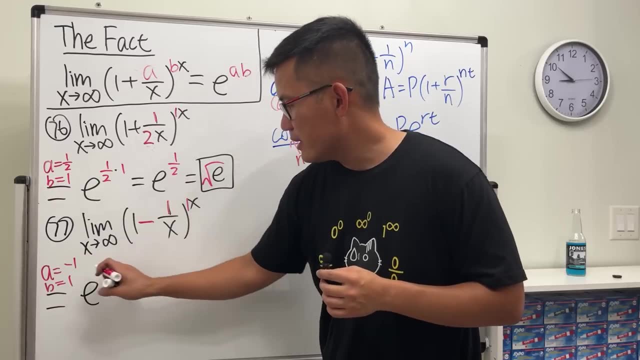 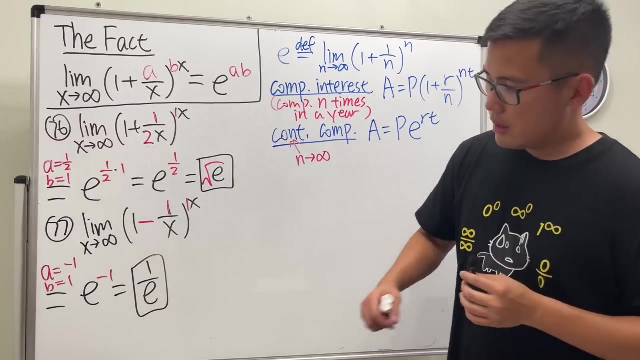 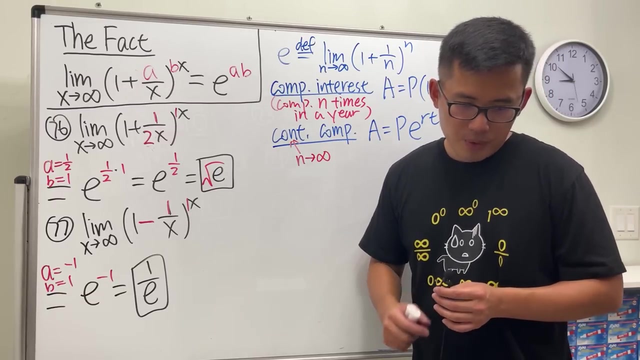 negative one, and then b is again one. so here, a is negative one and b is one. so it's e to the negative, one times one, which is negative one. so this is just one over e if you want to write it as a fraction, and if you want to write it as a rational form, one over e- okay, cool. 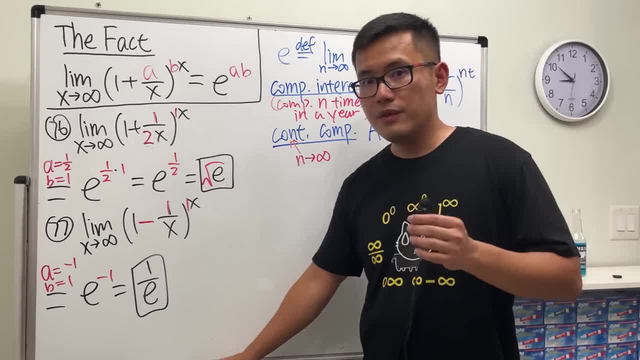 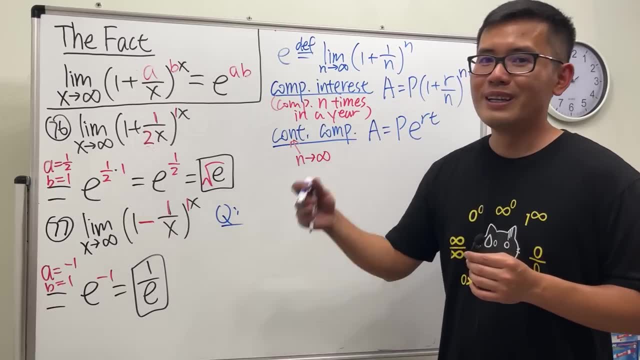 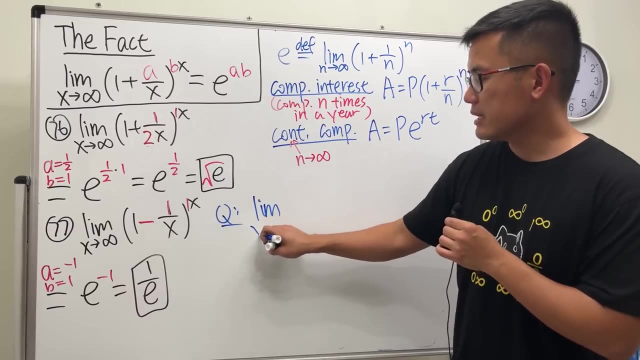 all right, i'm going to give you guys a question to see if you guys are really paying attention or not. question for you guys, all right. so leave a time stamp and also tell me what the answer is. you see how here is just x to the first power. what if we have the limit as x approaching infinity? 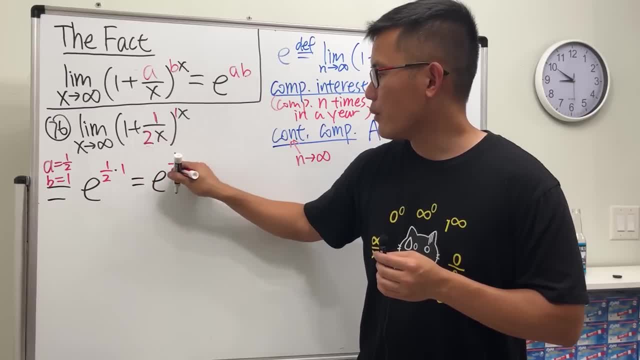 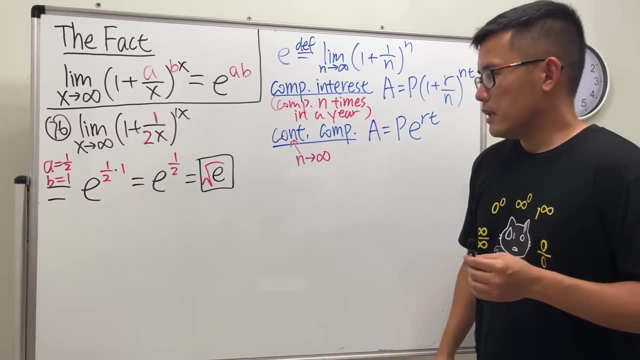 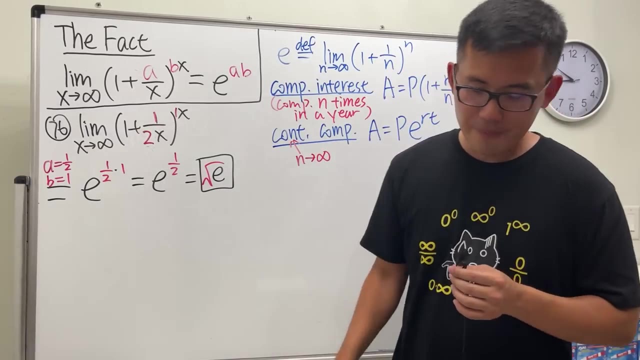 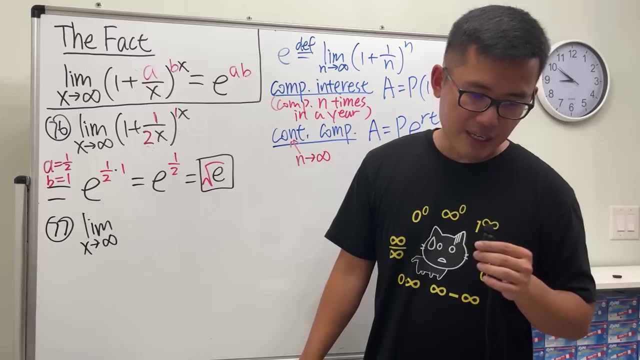 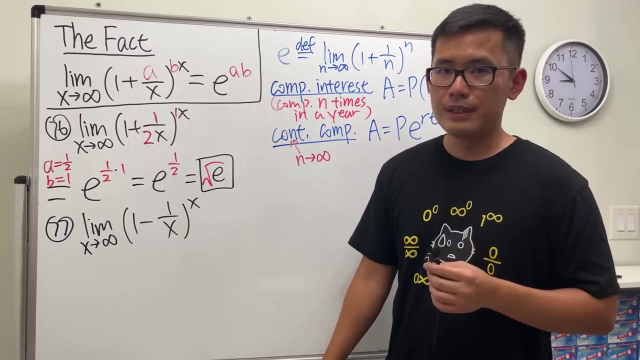 1, which is just e, to the 1 over 2 power, which is just the square root of e. all right, okay, so that's the answer for that, nice and quick. now try another one: 77 limit as x approaching infinity, and then we have 1 plus 1, minus this to the x power. so what's the? a value. 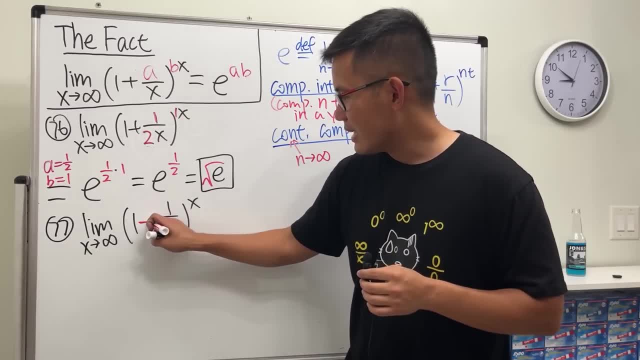 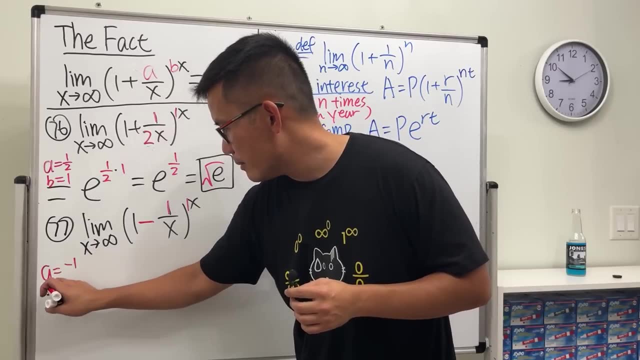 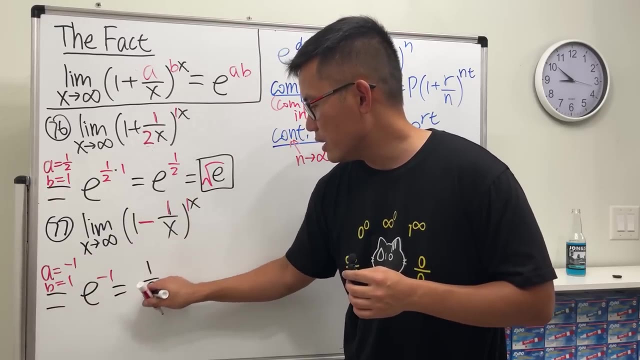 yeah, here negative 1. good, yeah, it's negative 1. and then b is again 1. so here a is negative 1 and b is 1. so it's e to the negative 1 times 1, which is negative 1. so this is just 1 over e, if you want to write it as a fraction. 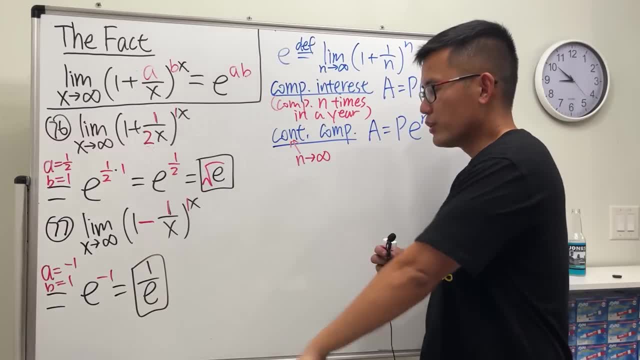 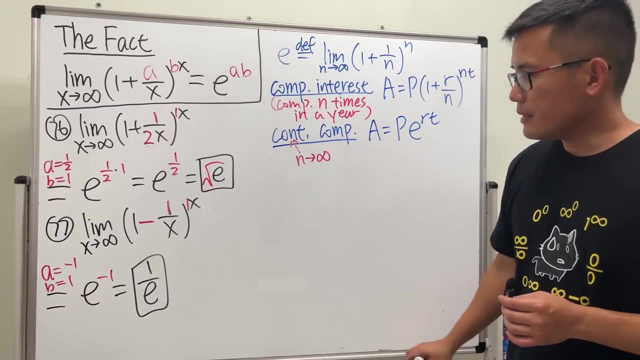 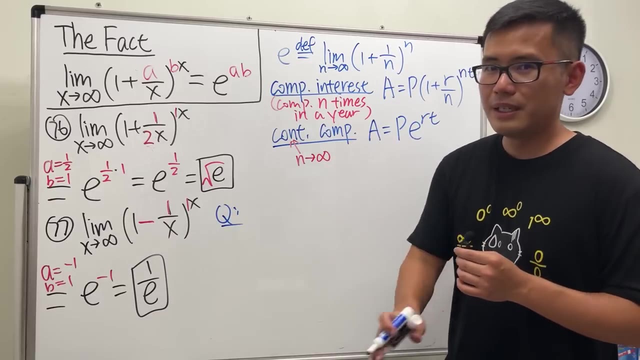 and if you want to write it as a rational form, 1 over e, okay, cool, all right, i'm going to give you guys a question to see if you guys are really paying attention or not. question for you guys, all right. so leave a comment below and i'll see you in the next video. bye, bye. 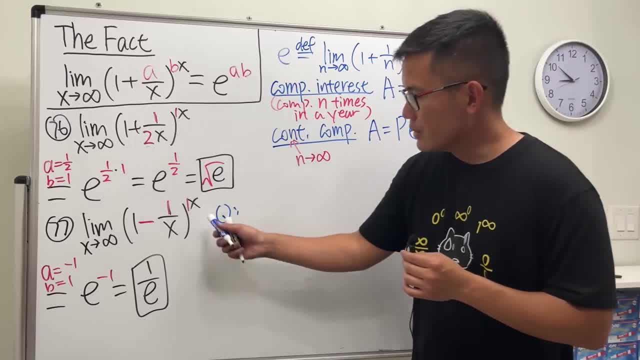 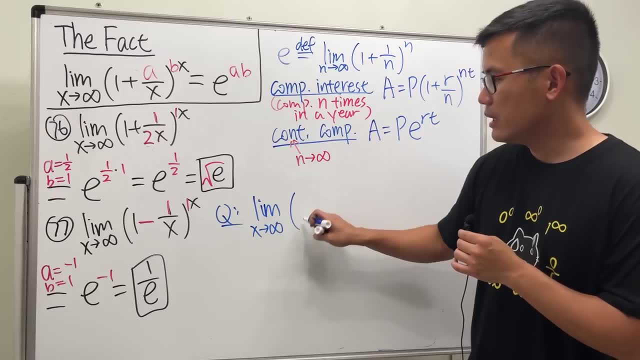 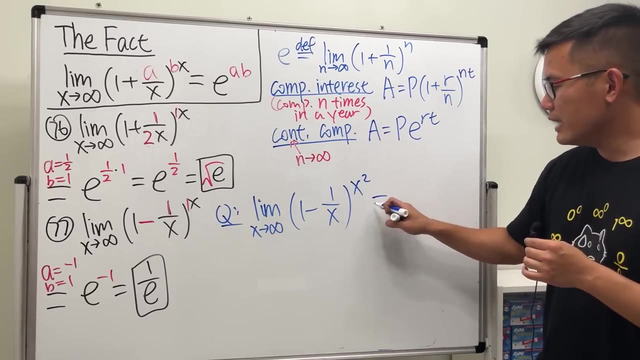 times them and also tell me what the answer is. you see how. here is just x to the first power. what if we have the limit as x approaching infinity, 1 minus 1 over x and then raised to the x square power? go ahead, think about this and then let me know what the answer is in the comment down. 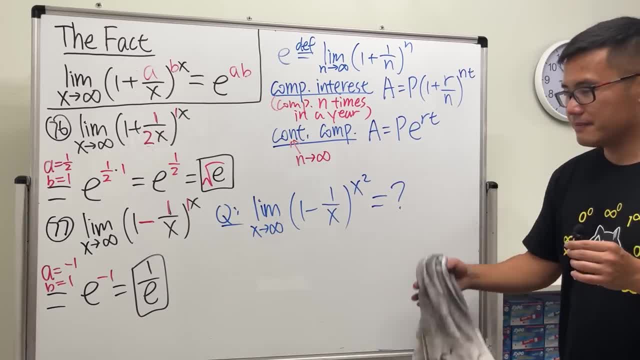 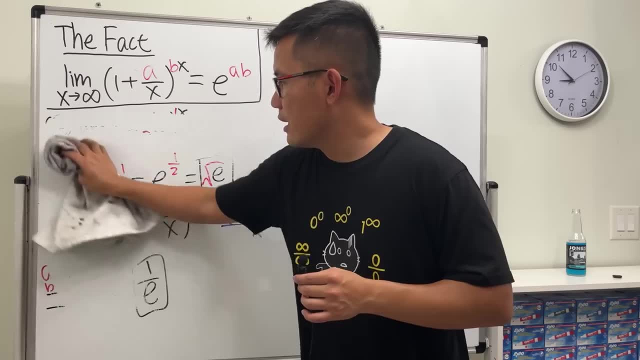 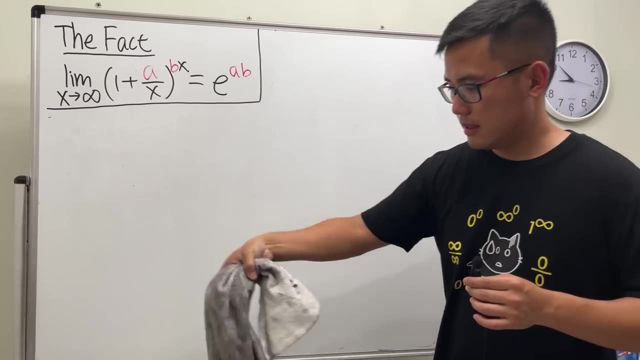 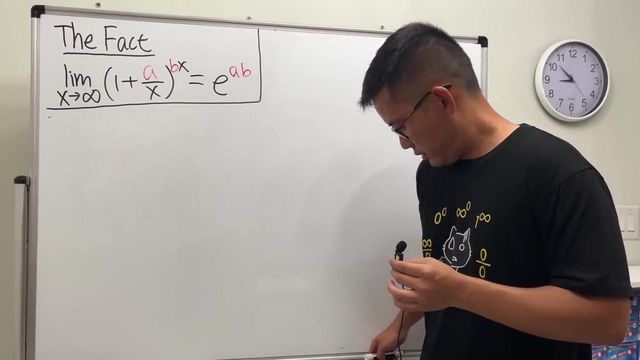 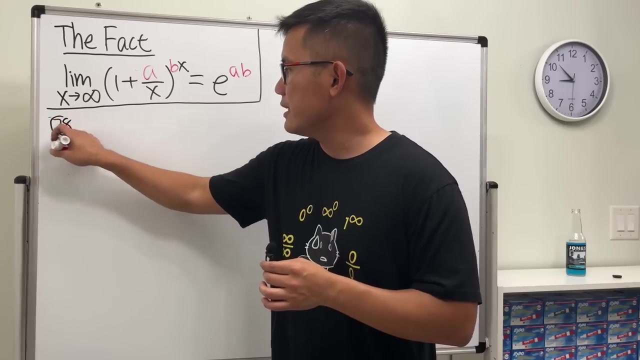 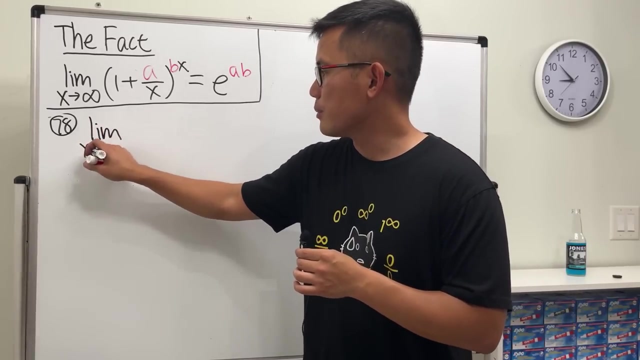 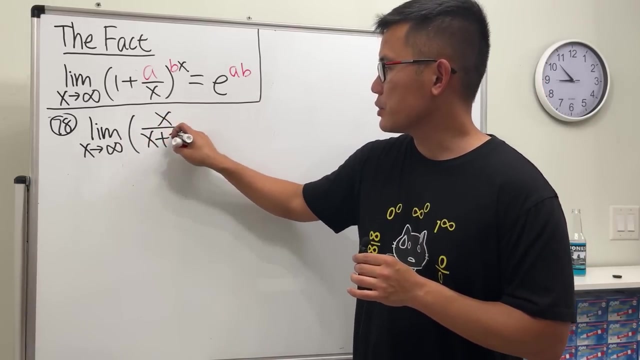 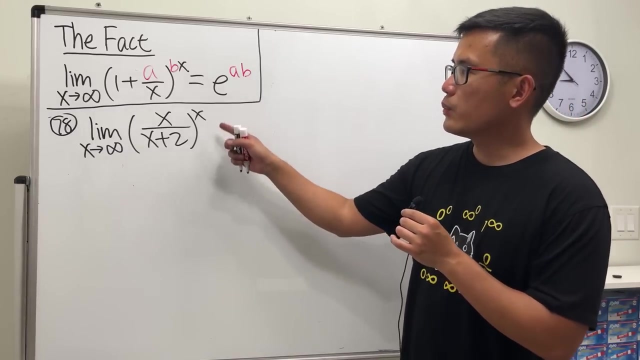 below: all right, okay, all right. number 78: okay it as x approaching infinity. and then we have- oh, this is different- x over x plus 2 raised to the x power. okay, so how do we do this? well, again, we are going to utilize the fact, and this is how. 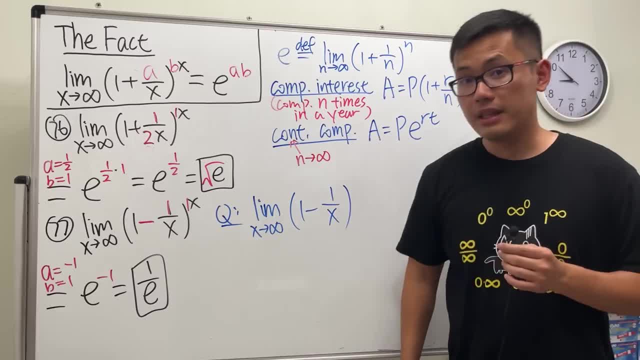 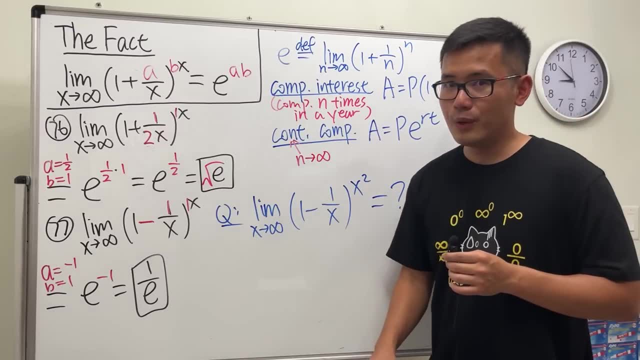 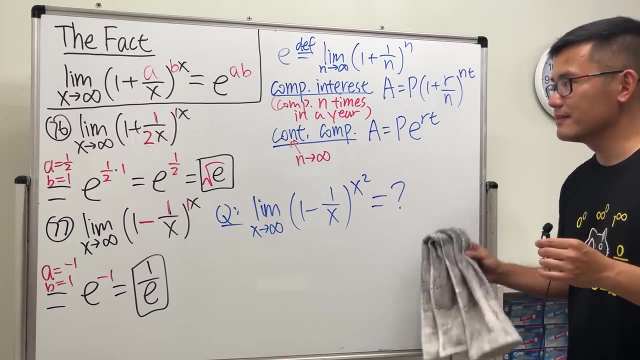 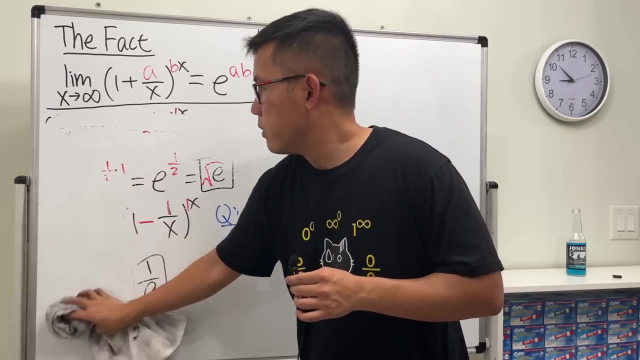 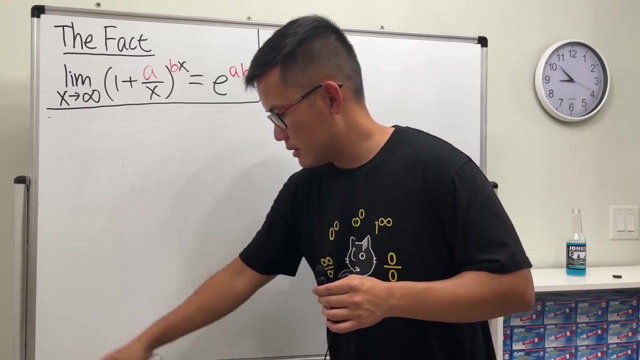 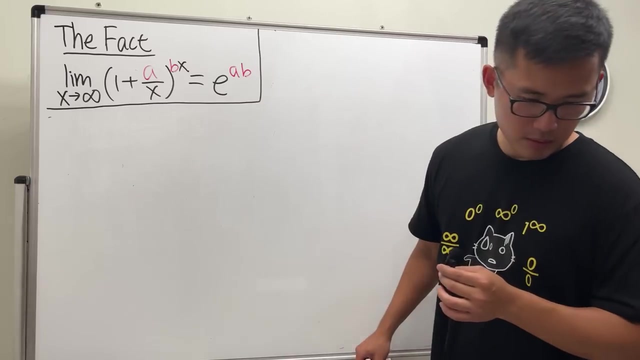 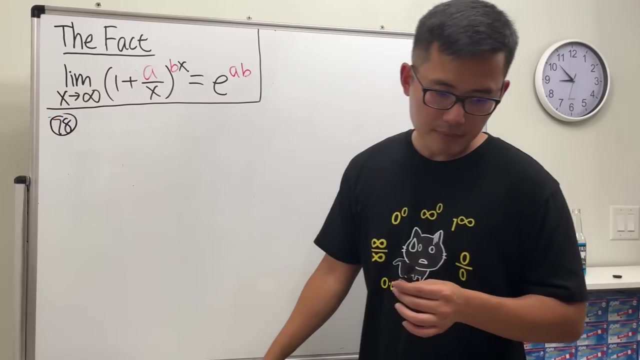 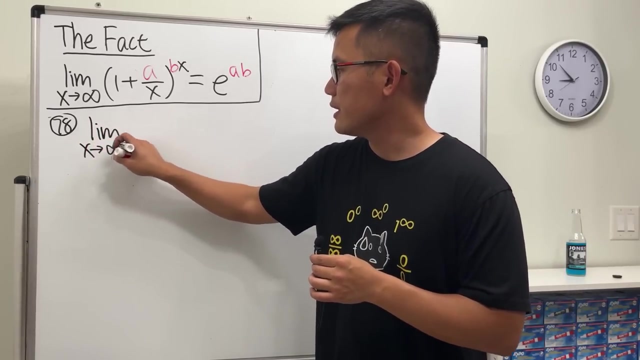 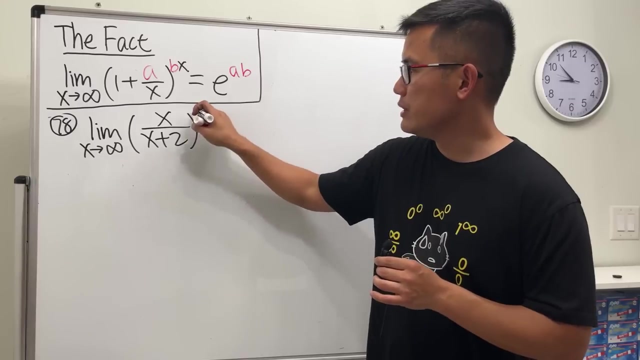 1 minus 1 over x and then raised to the x squared power. go ahead, think about this and then let me know what the answer is in the comment down below. all right, okay, all right. number 78: limit as x approaching infinity. and then we have- oh, this is different- x over x plus 2 raised to the 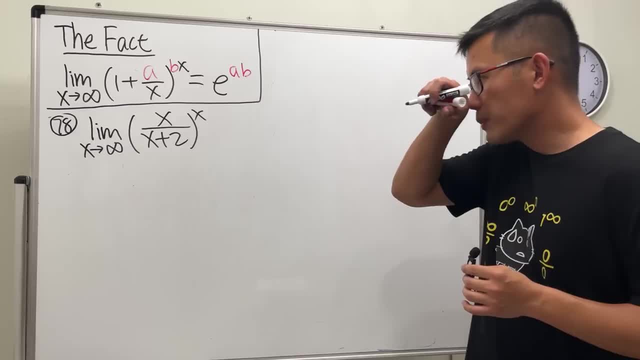 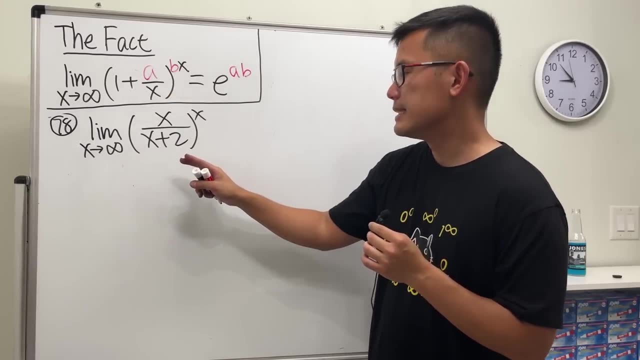 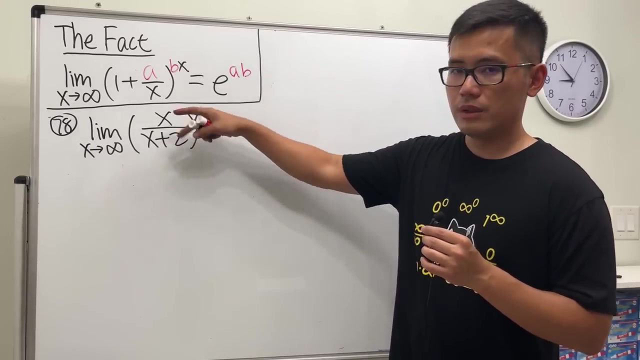 x power. okay, so how do we do this? well, again, we are going to utilize the fact, and this is how: first, we see that we have two turns on the bottom. we don't like that, because we cannot split the fraction easy this way, right, so why don't we kind of just flipped it? can we do that? yes, we just have. 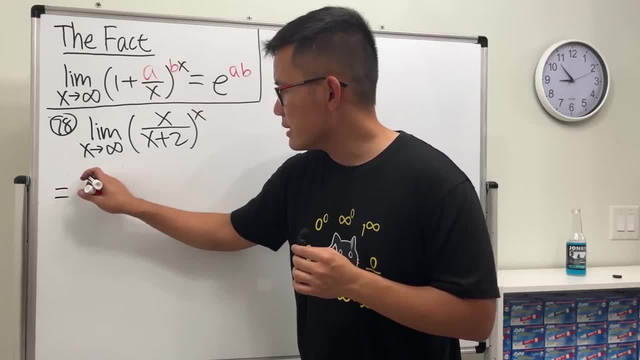 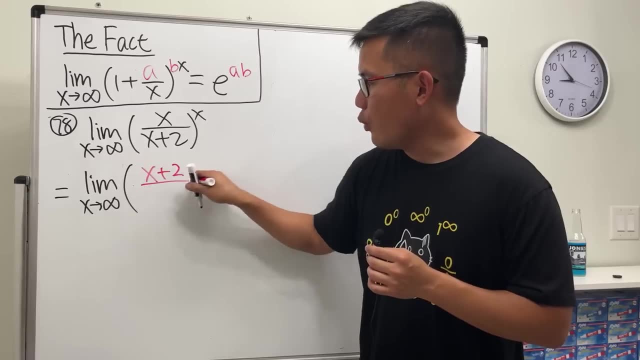 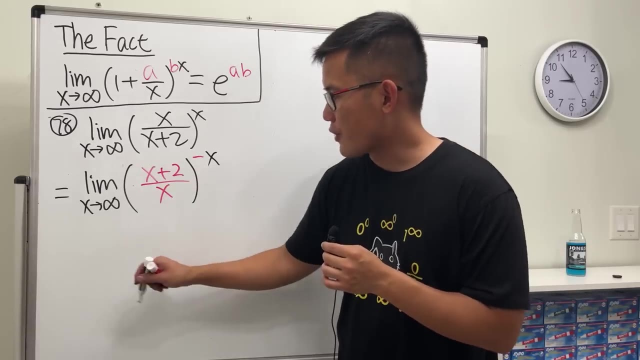 to negate the power. so let's go ahead and write this as the limit as x approaching infinity and then for the inside i'm going to put it as x plus 2 over x and then raised to the negative x power. aha, and now we can split the fractions. so we are looking at the limit as x approaching infinity. 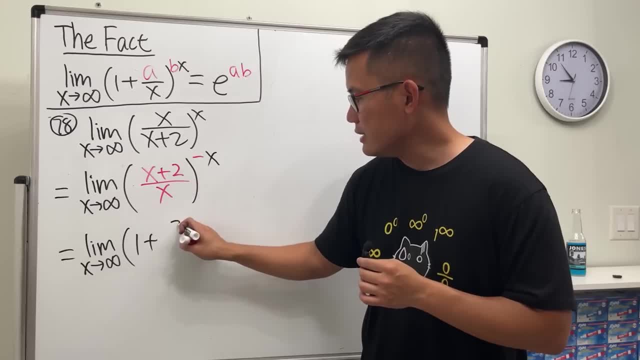 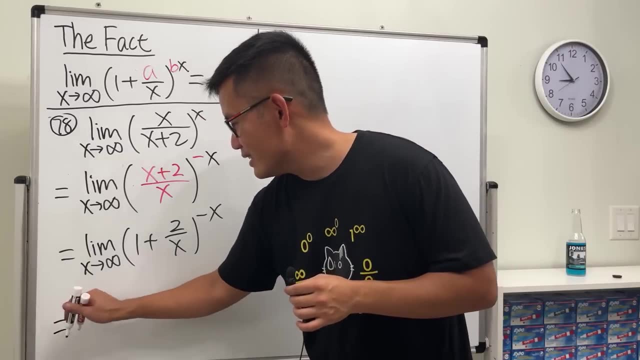 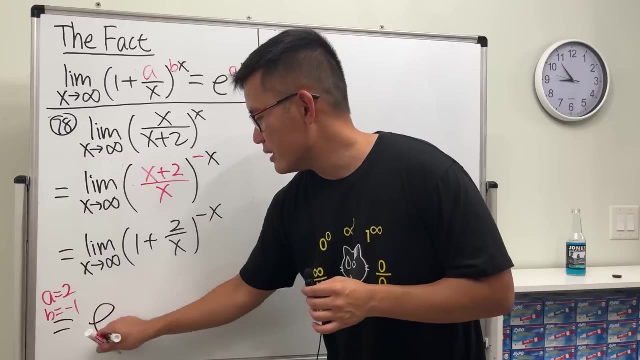 and then this is 1 plus, this is 2 over x and then minus x. so a is equal to 2, b is equal to negative 1. all together is e to the, this times that which is negative 2 and if you would like, you can write it as 1 over. 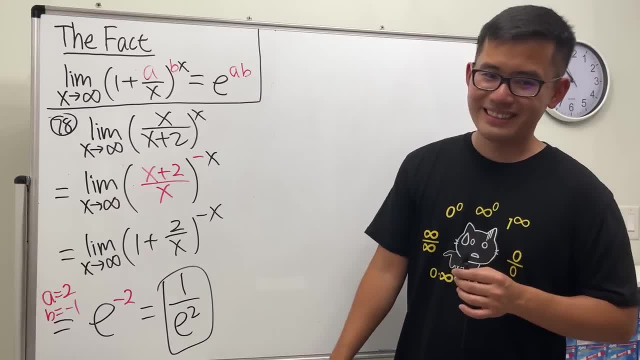 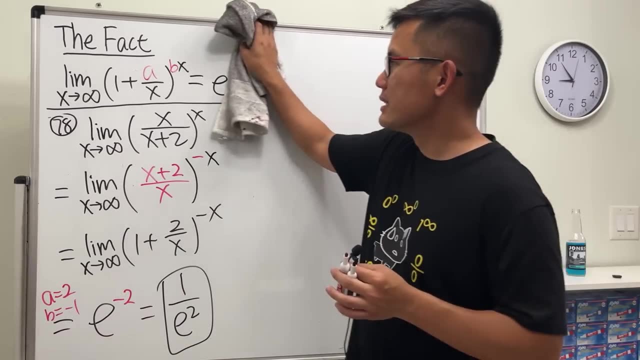 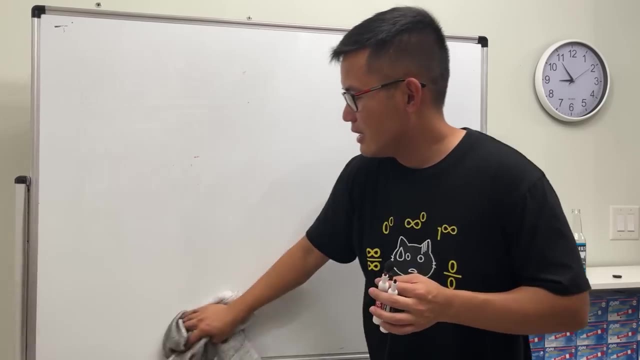 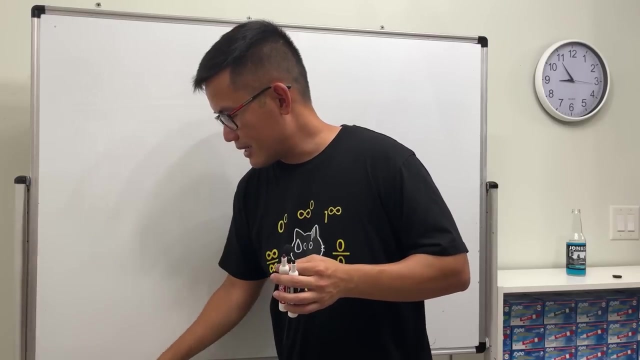 e squared, and then we are done. cool huh, all right. so this is the fact for that, and now i will show you guys the limit, which is the one that caused a lot of argument too, for limits. lapito's rule will not, lapito's rule will, or not? 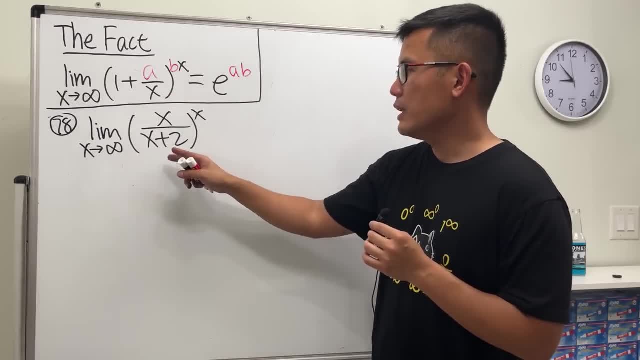 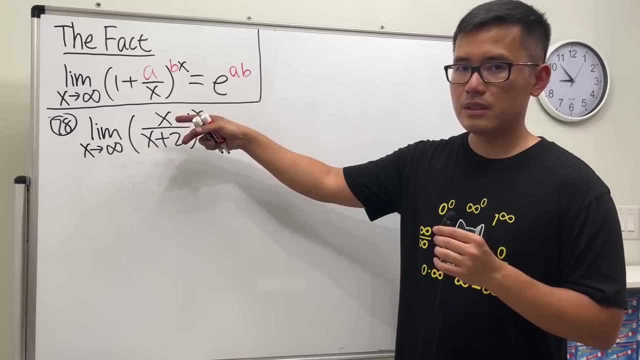 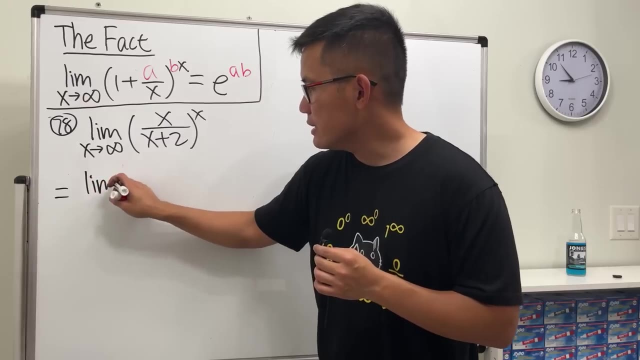 first, we see that we have two turns on the bottom. we don't like that, because we cannot split the fraction easy this way, right? so why don't we kind of just flip it? can we do that? yes, we choose how to negate the power. so let's go ahead and write this as the limit, as x approaching infinity and 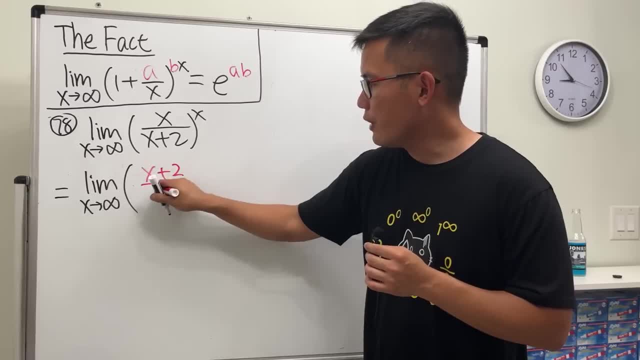 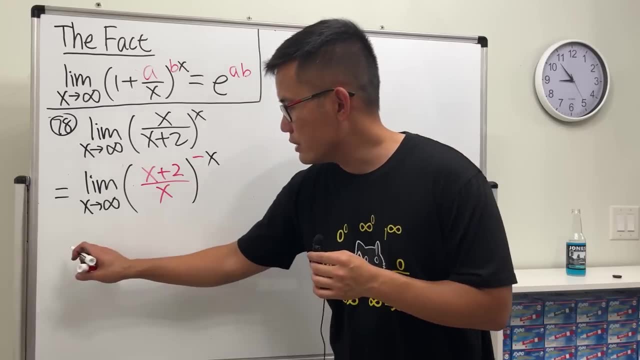 then for the inside, i'm going to put it as x plus 2 over x, and then raised to the negative x power. aha, and now we can split the fractions. so we are looking at the limit as x approaching infinity, and then this is 1. 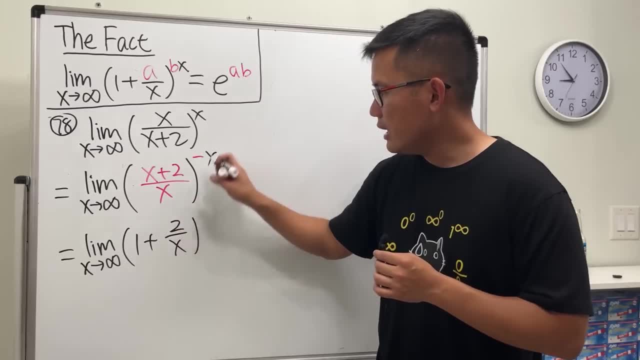 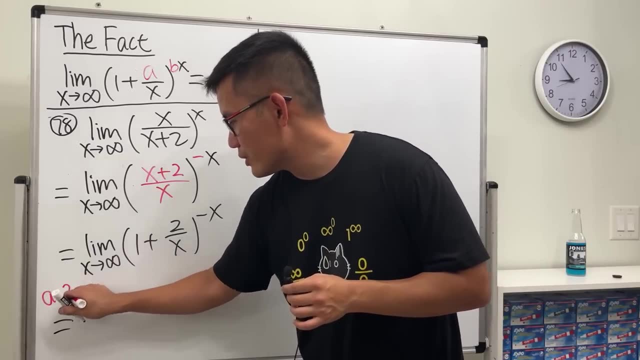 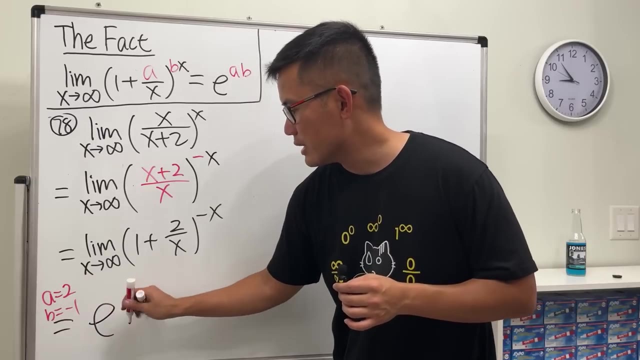 plus this is 2 over x and then minus x, so a is equal to 2, b is equal to negative 1. all together is e to the, this times that which is negative 2, and if you would like, you can write it as 1 over e squared, and then we are done. 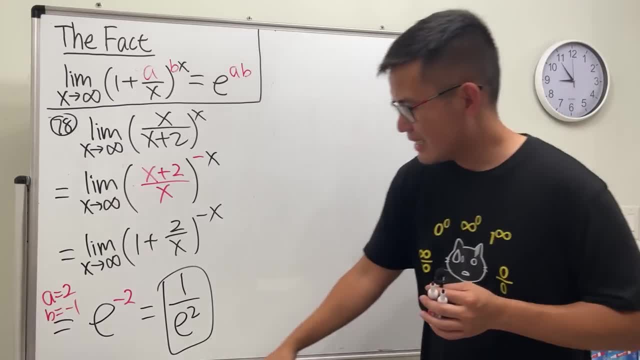 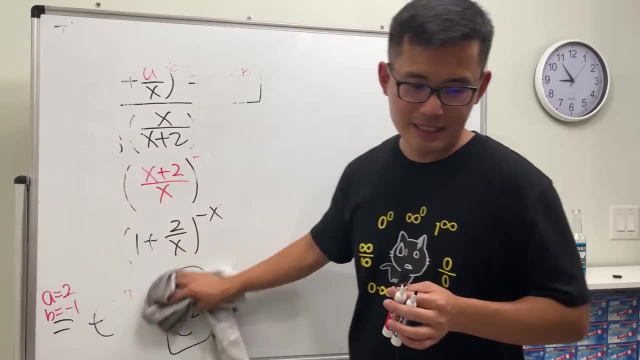 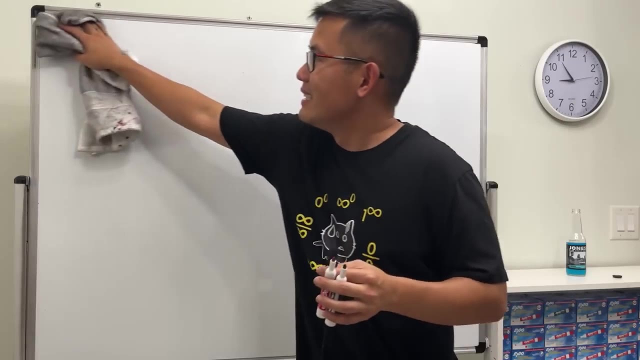 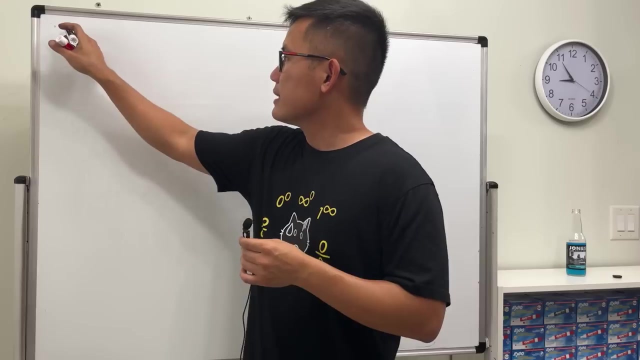 cool, huh, all right. so this is the fact for that, and now i will show you guys the limit, which is the one that caused a lot of argument too for limits. labrador's rule will not labrador's rule work, or not all right. so this right here, i call this the limit. 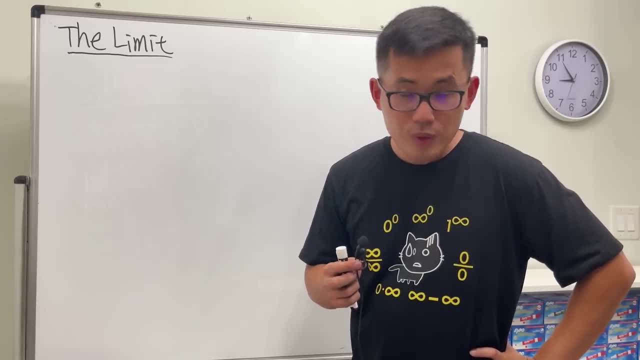 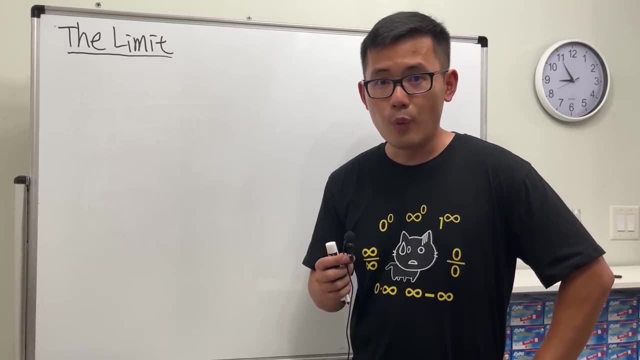 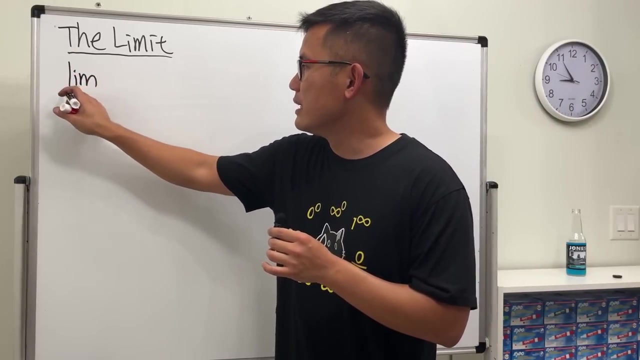 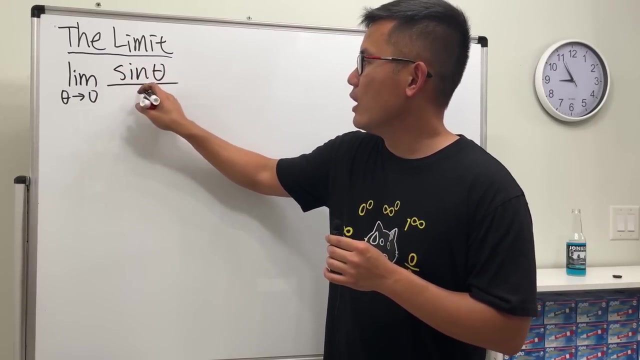 so you see, a lot of time we have 100 and one 100 something limits already and, uh, why is this one, the one i call the limit, right? yeah, anyway, i'm going to use theta for it. this is the limit as theta approaching zero and we are going to get sine of theta over theta and this is equal to one. 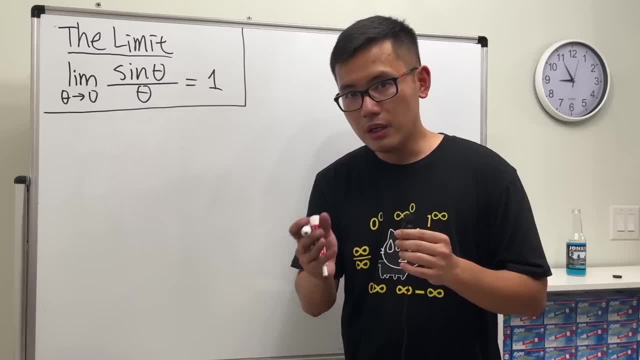 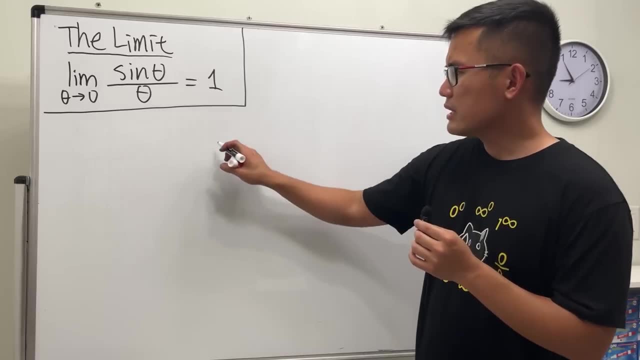 this is the limit. why? because earlier we talked about the labrador's rule and you see that if theta is equal to zero, then we get zero for zero. so it looks like hey to do this. it's super easy, because when we have the limit as theta, 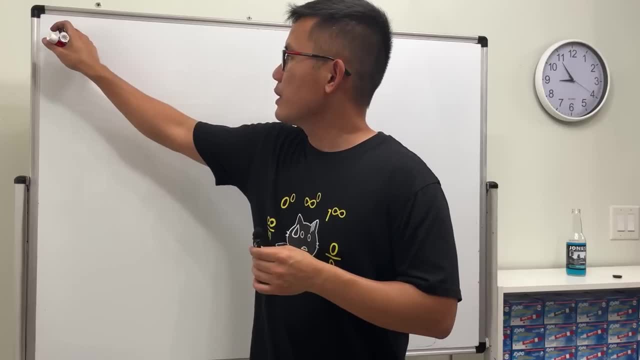 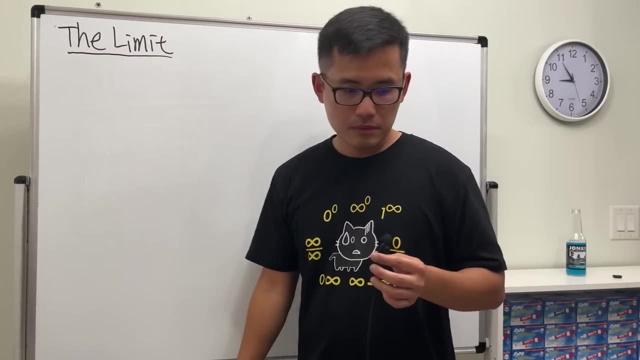 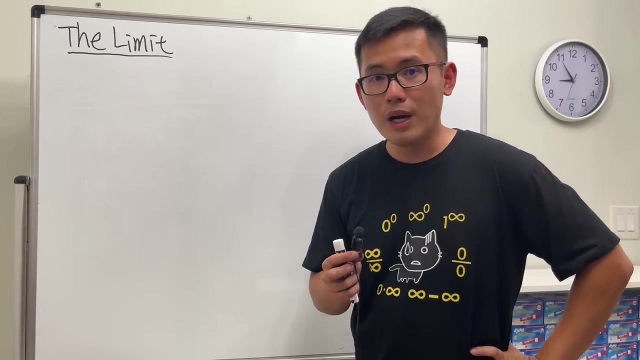 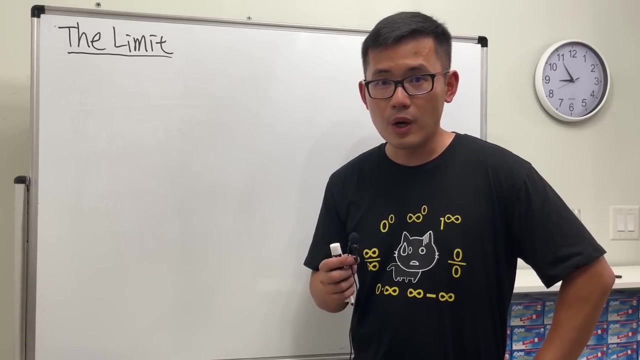 all right. so this right here, i call this the limit. so you see, a lot of time we have 100 and one more 100 something limits already and, uh, why is this one, the one i call the limit, right? yeah, anyway, i'm going to use you. 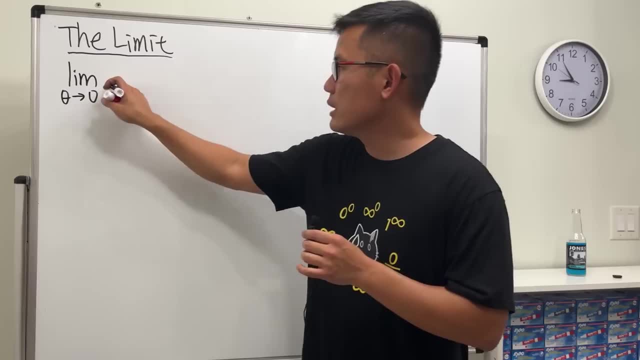 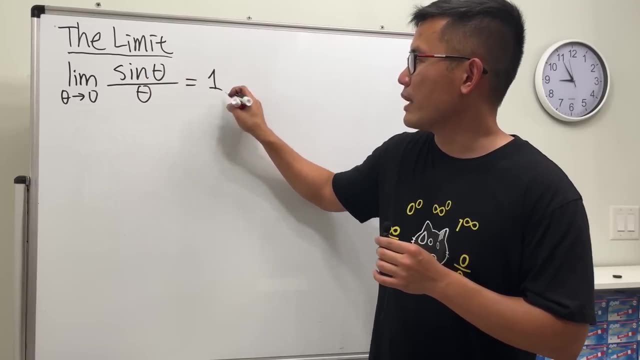 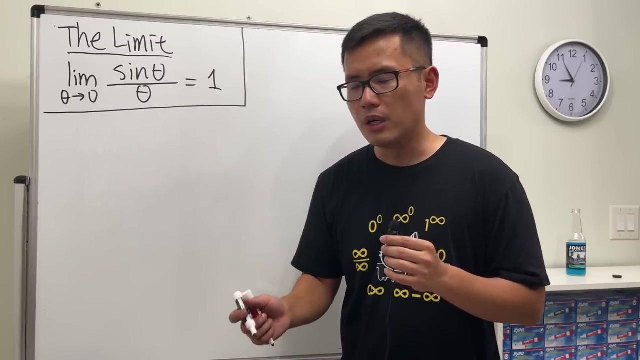 data for it. this is the limit, as theta approaching zero and we are going to get sine of theta over theta and this is equal to one. this is the limit why? because earlier we talked about the lapido's rule and you see that if theta is equal to zero, then we get zero for zero right. 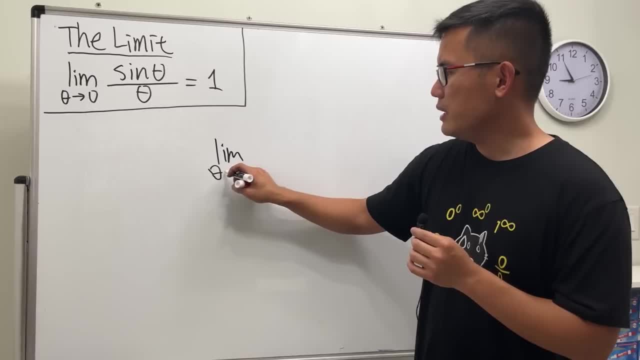 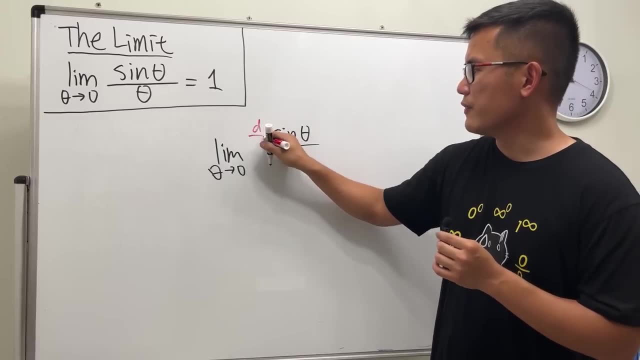 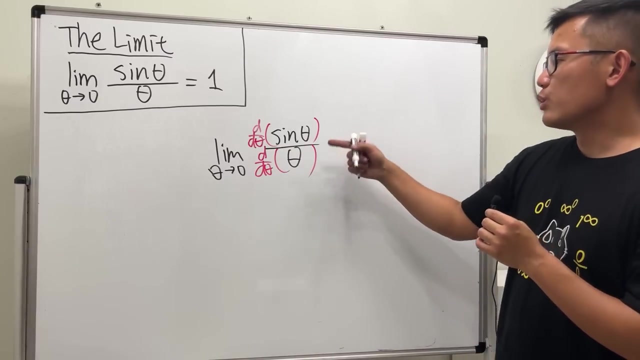 so it looks like, hey, to do this is super easy, because when we have the limit as theta approaching zero, we can just go ahead and do the lapito's rule. let's go ahead and differentiate this with respect to theta and then do the same thing as well. wow, and you see the derivative of this. 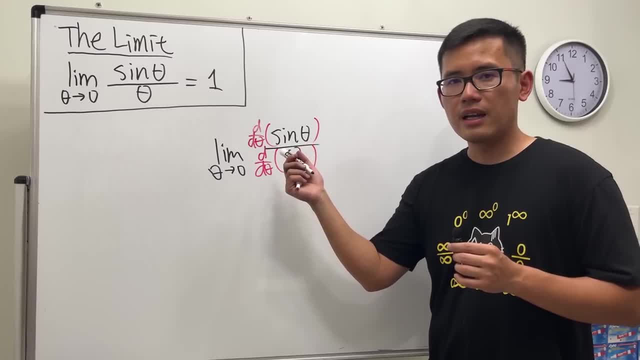 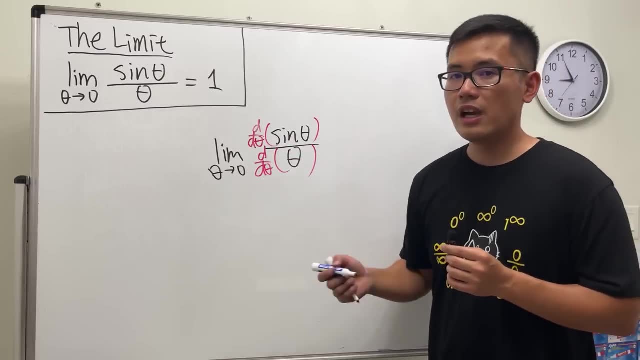 well, what's that? what's the derivative sine theta? yes, you can tell me cosine, but how do we do it? well, if you recall the way that we did the derivative of sine of x, uh, you will recognize that when we are saying: well, if we do infinite sigma, x, weight, of course you some say the derivative of sine delta and zero of x. so helicopter power will not work. however, if we do linear equilibrium, carro deal equals to zero, power will honor matrix work and then loveing is equal to sigma and the argument for love. 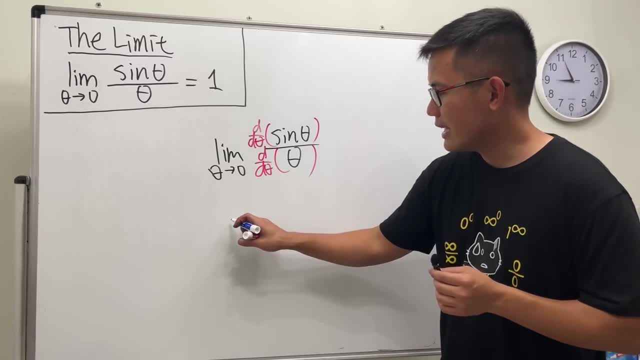 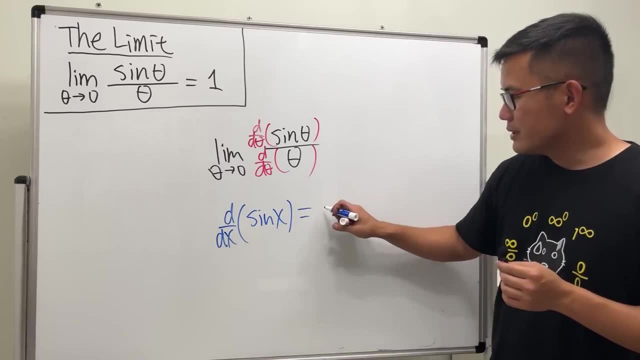 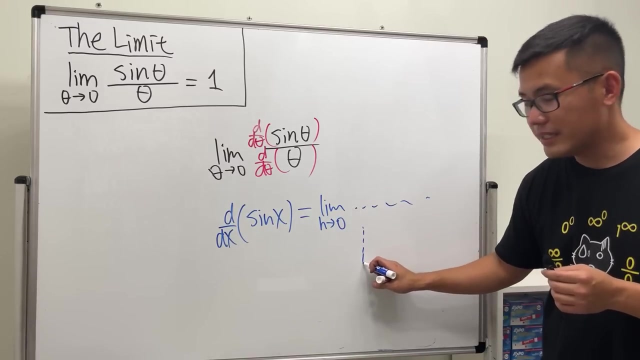 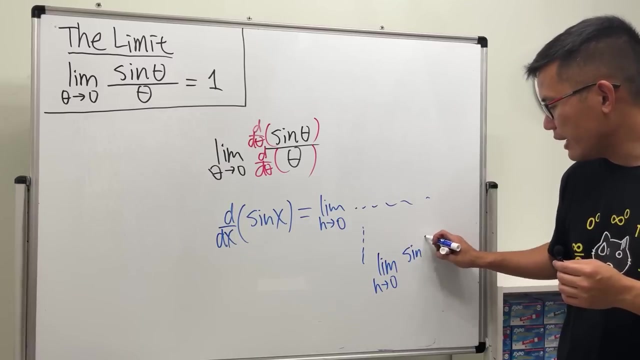 ahor doing the derivative of sine x. all right, you use the. we will use the definition of derivative, the limit as x approach h approaches zero, all the stuff, all the stuff, right. and then somewhere we have what? the limit as h approaching zero, sine of h over h. and here we are using the h for the. 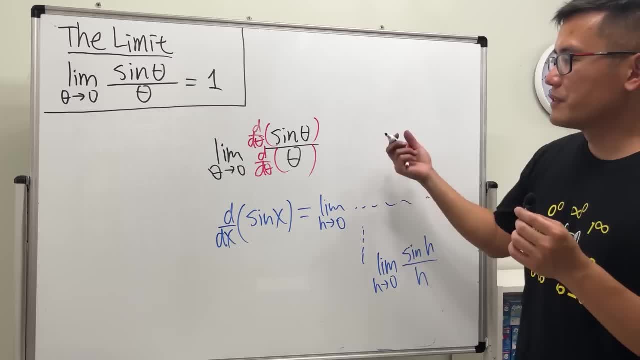 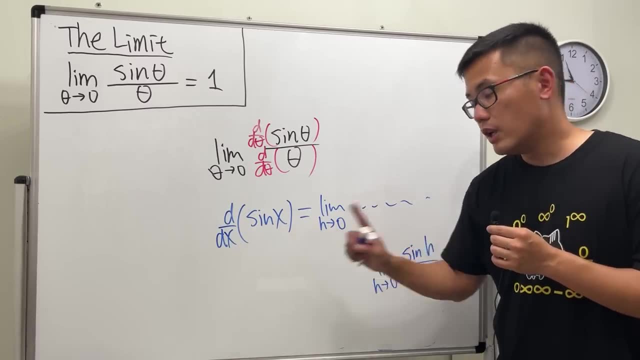 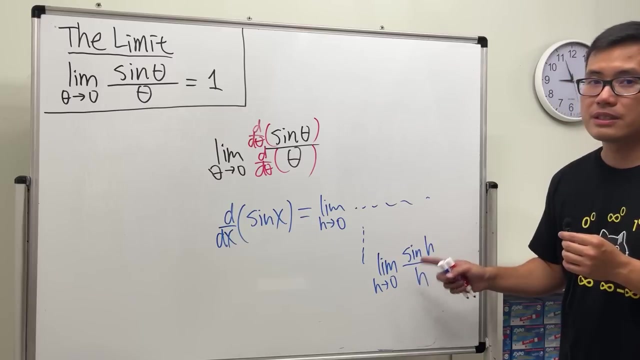 variable. you cannot just change your variable and then, all of a sudden, you know how to take the derivative. no, you see, in order for us to use, in order for us to get the derivative of sine x, we will have to find the. uh, we will have to find the. we will have to find this limit first. 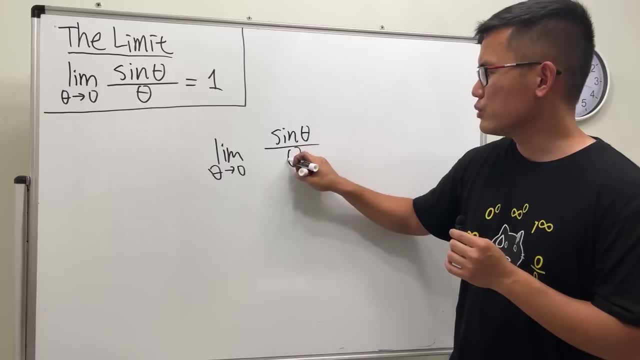 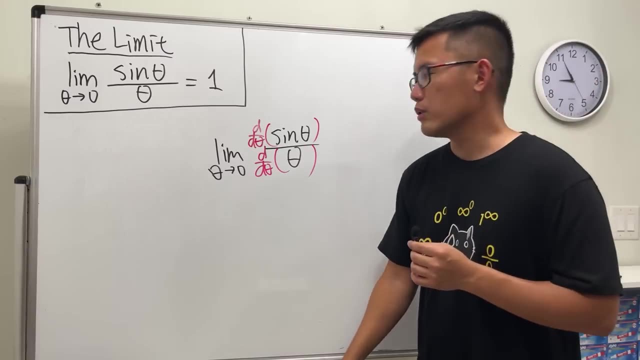 approaching zero. we can just go ahead and do labrator's rule like, go ahead and differentiate this with respect to theta and then do the same thing as well. wow, and you see the derivative of this vote. what's that? what's the derivative of sine theta? 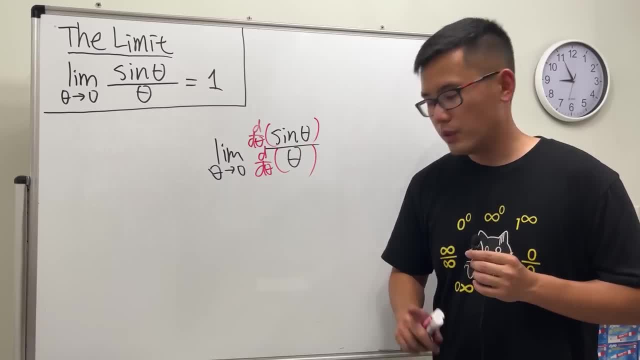 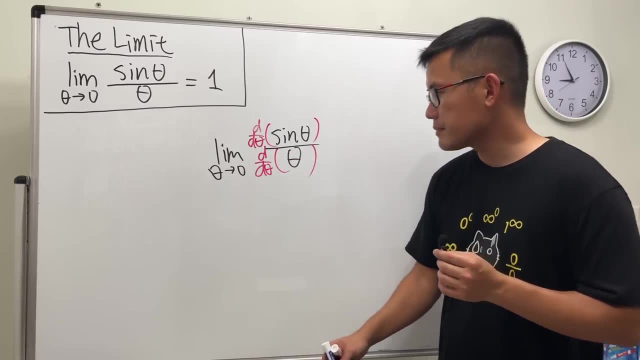 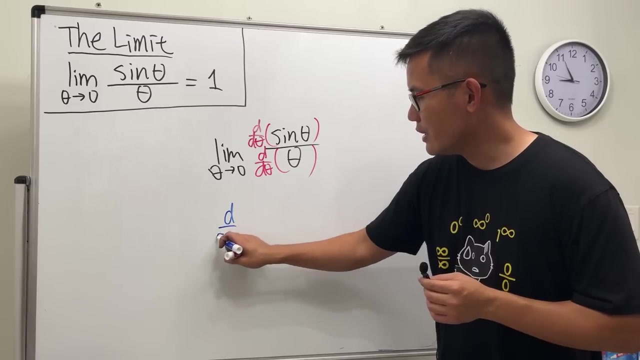 yes, we can do the same thing several times here. what is the derivative of sine theta? and yes, you can tell me cosine, but how do we do it? well, if you recall the way that we did the derivative of uh, something that sine of x, uh, you will recognize that when we are doing the derivative of 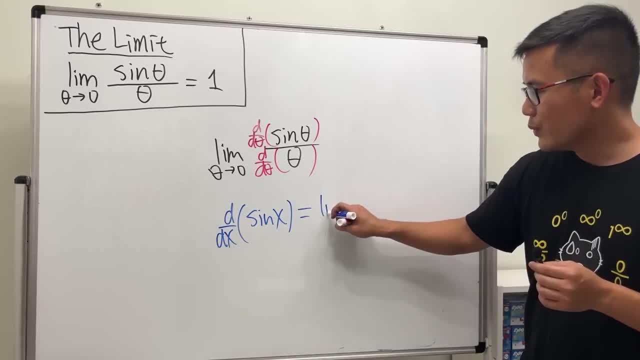 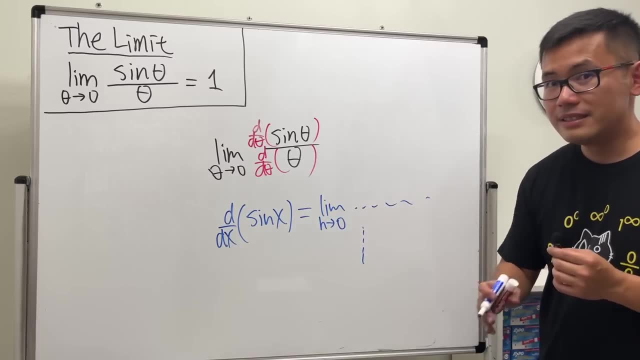 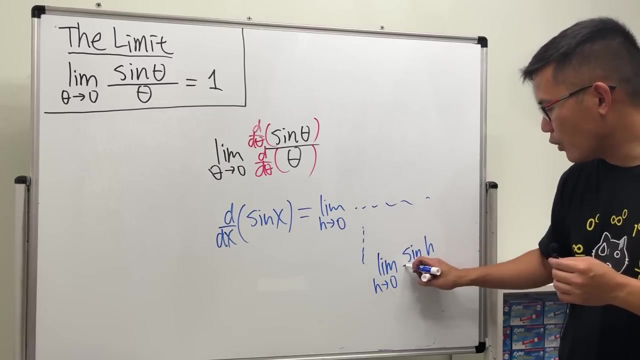 sine x. all right, you use the we, we use the definition of derivative, the limit as x support: h approaches zero. all the stuff, all the stuff, right. and then somewhere we have what? the limit as h approaching zero, sine of h over h. and here we are using the h for the variable. 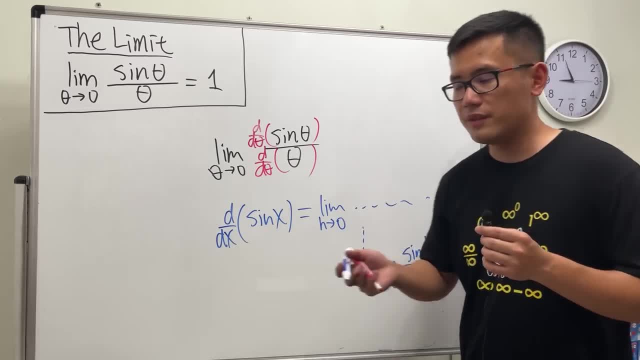 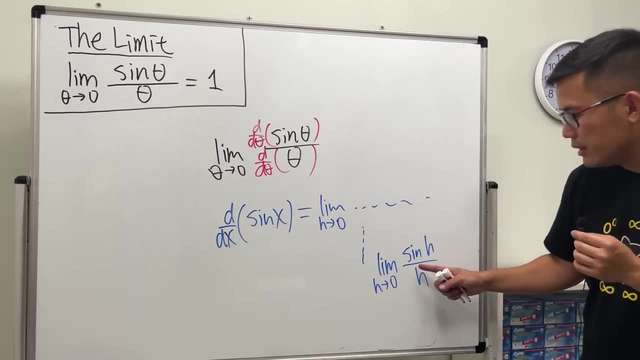 you cannot just change a variable and then, all of a sudden, you know how to take the derivative. no, you see, in order for us to use, in order for us to get the derivative of sine x, we will have to find the. uh, we will have to find the. 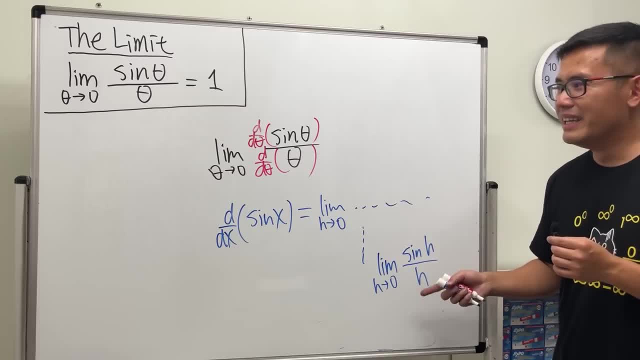 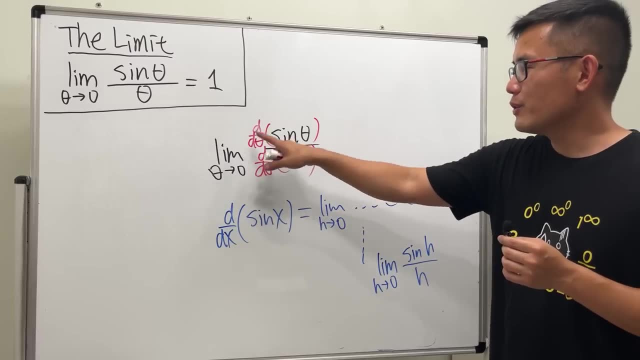 we will have to find this limit first. but how can we use the? how can we use the derivative? right now? if i'm trying to use, if i'm trying to find this limit, how can we find it? how can we use the derivative? we cannot. so this: 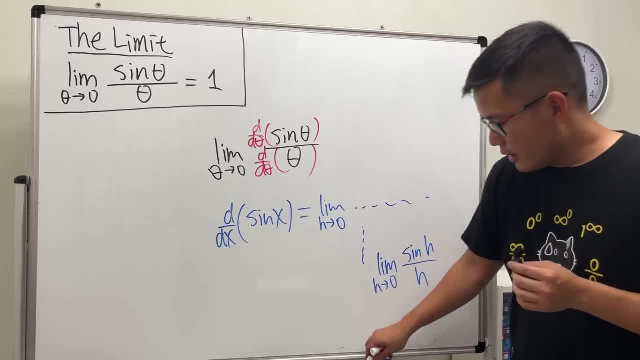 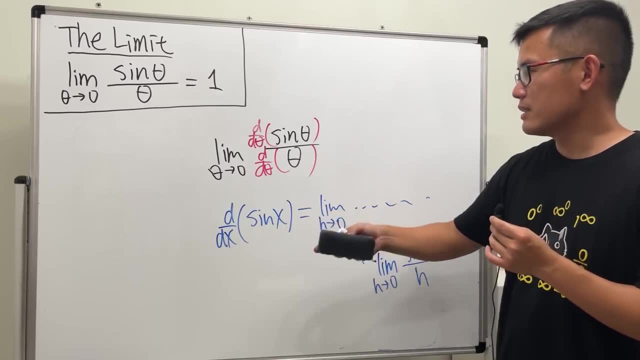 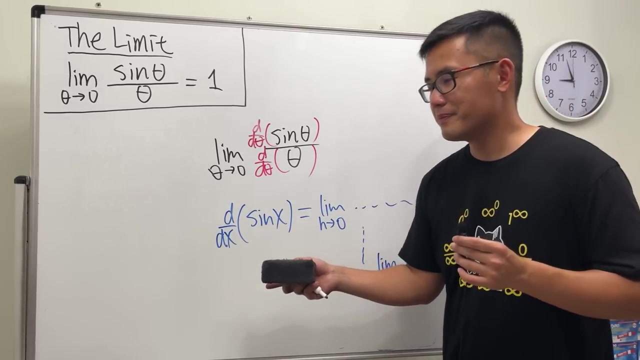 is called circular reasoning. yeah, so a couple ways to fix this one. you can use numerical method, meaning i just use, uh, the table of values plug-in, you can see the answer. you know is equal to one. or you can do a geometric proof, which i didn't do, yeah, but i give you guys a graphical proof. i graph. 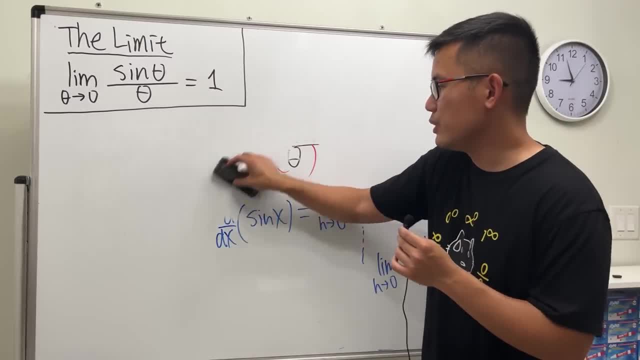 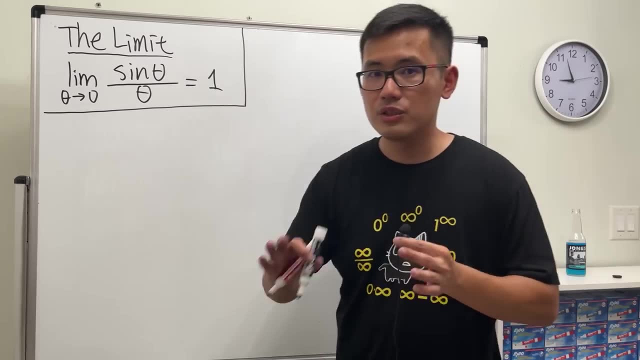 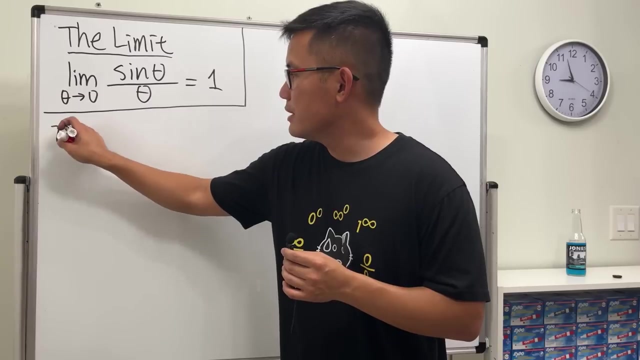 sine x over x, and we saw that the limit of this is equal to one. but here i have something better. whenever you encounter this kind of limits, just say by the limit, and then the answer is one and we are done here. number 79: let me show you how we can work this out. 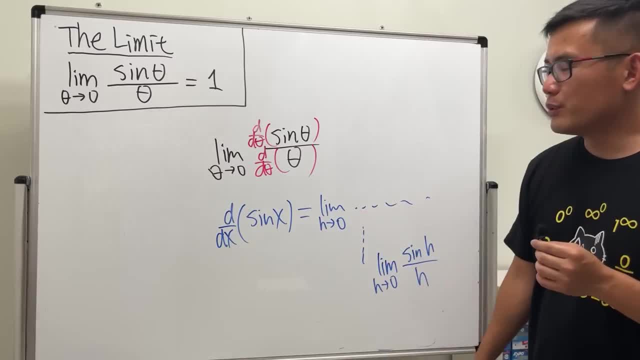 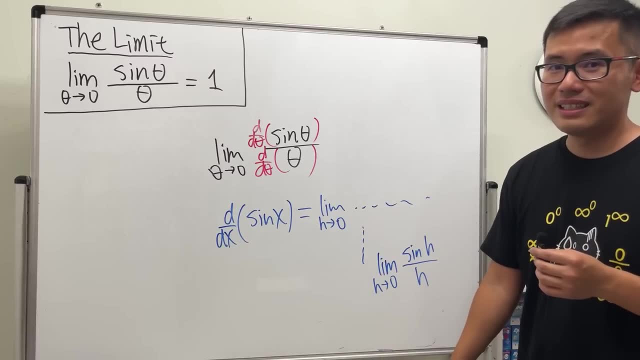 but how can we use the devin? how can we use the derivative? right now, if i'm trying to use, if i was trying to find this limit, how can we find it? how can we use the derivative? we cannot, so this is called circular reasoning, yeah, so. 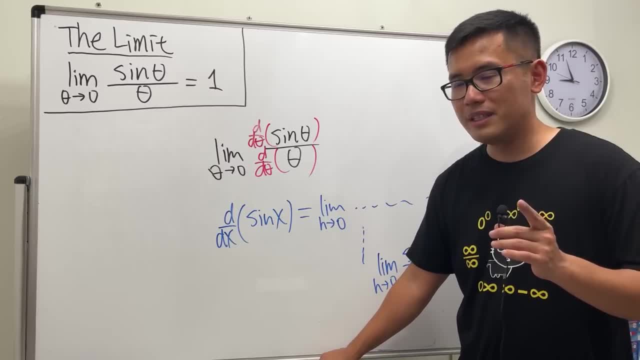 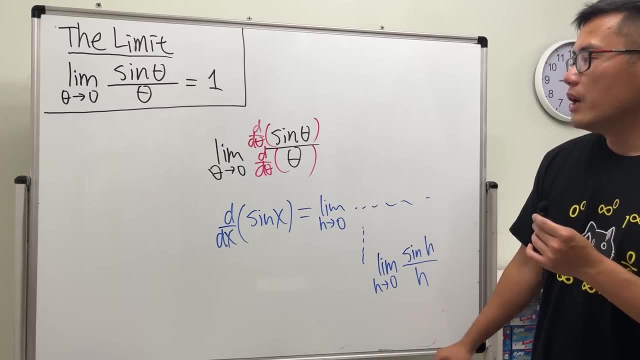 a couple ways to fix this one. you can use numerical method, meaning i just use a, the table of values plug-in, you can see the answer. you know is equal to one. or you can do a geometric proof, which i didn't do, yeah, but i give you guys a graphical proof. 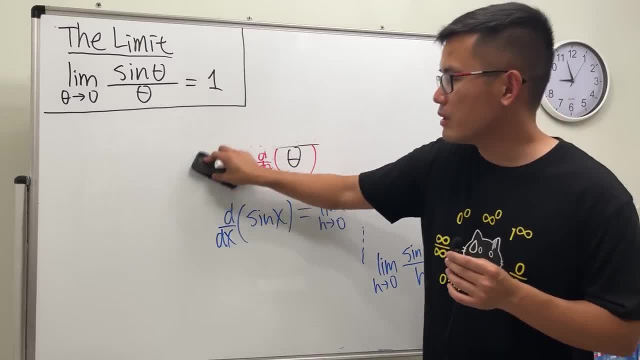 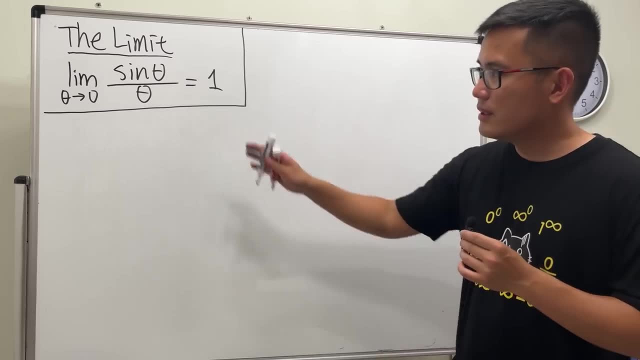 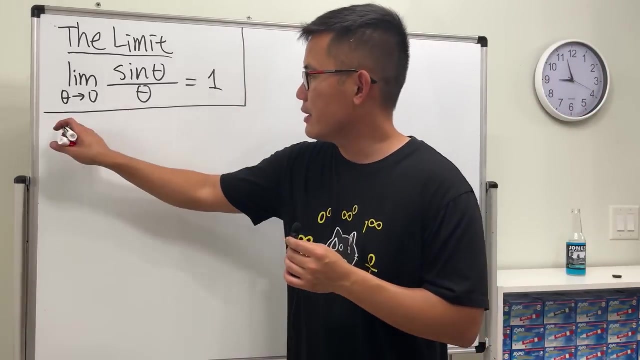 i graphed sine x over x and we saw that the limit of this is equal to one. but here i have something better. whenever you encounter this kind of limits, just say by the limit that? um, the answer is one and we are done here. number 79: let me show you how we can work this out. 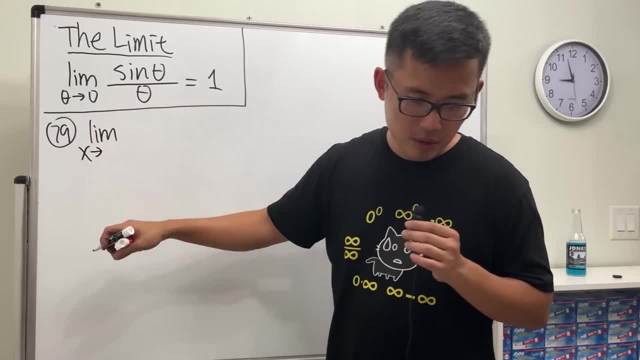 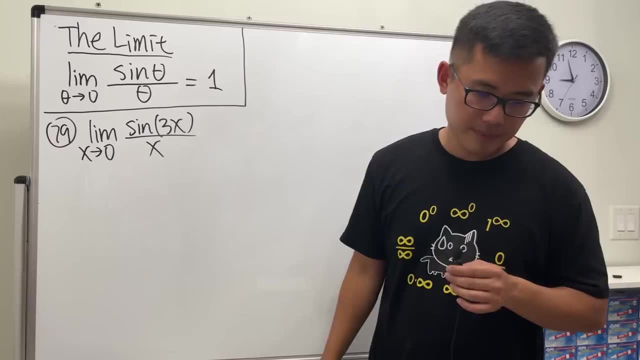 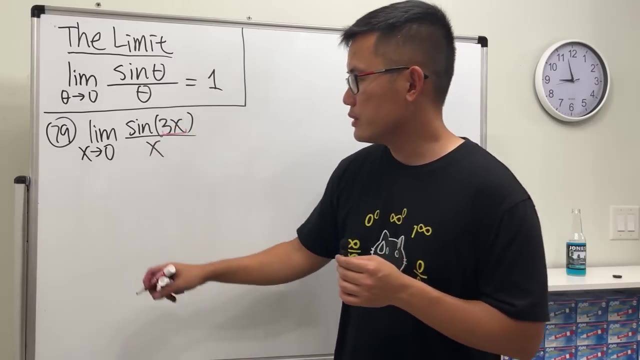 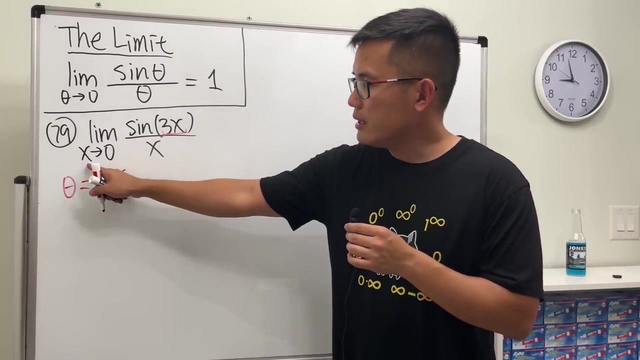 limit as x approaching zero. and then we have sine of 3x over x. okay, here the input is 3x. what we can do is just do a nice substitution: call theta to be 3x and you see, when x is approaching 0, you can put it here: 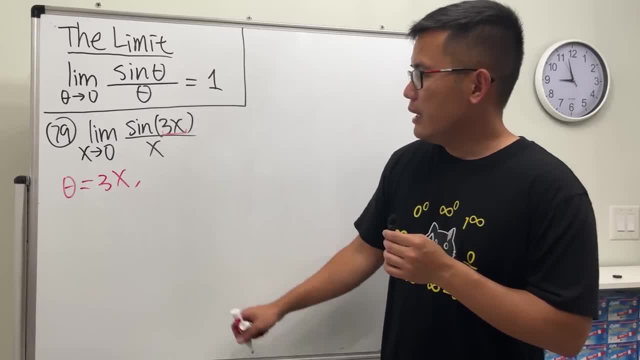 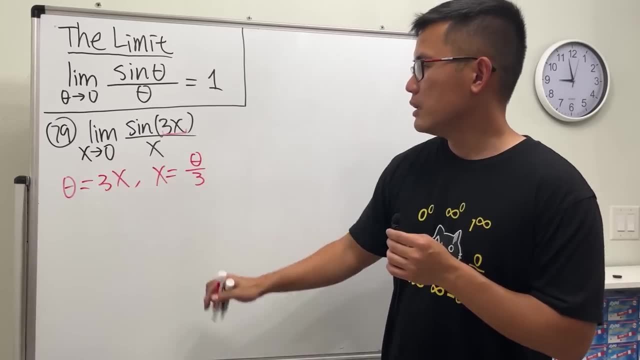 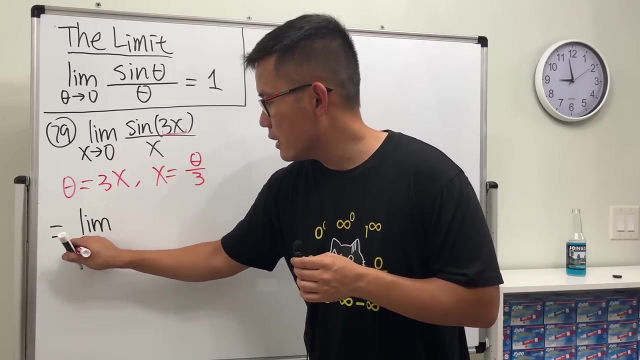 theta is approaching 0 as well. good, and perhaps we can also solve for x. we can divide the 3 on both sides. this means x is equal to theta over 3. so you can see, this is going to be the limit. but x approaching 0 implies theta will go to 0, and then here we have sine and then this right. 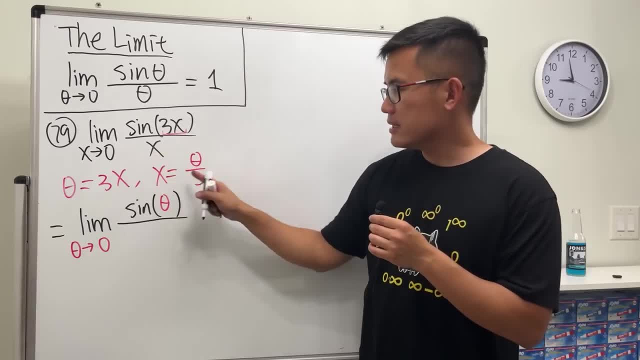 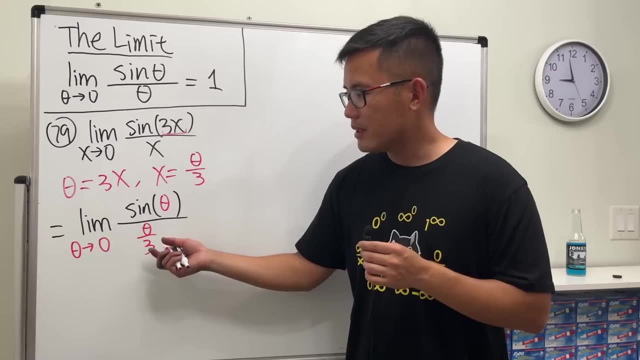 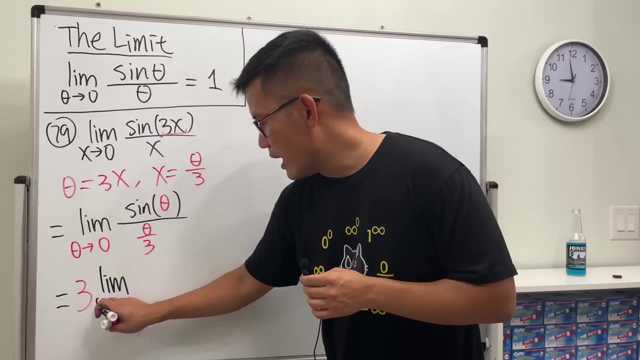 here is theta inside now, and then the x is theta over 3, but you know the over 3 in the denominator we can put it up right here. so all in all we can say this right: here is 3 times the limit as theta going to 0 and then x is going to be 0. 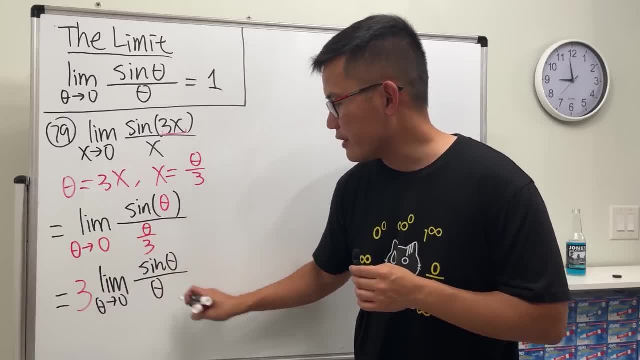 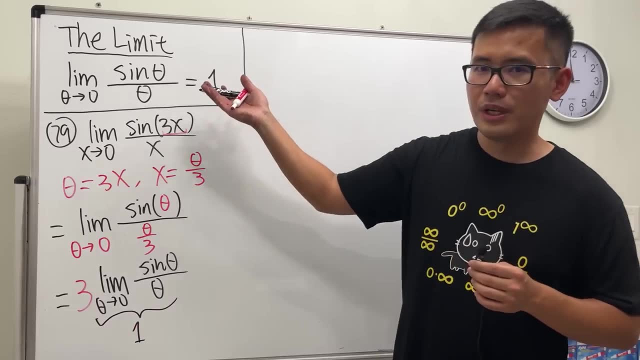 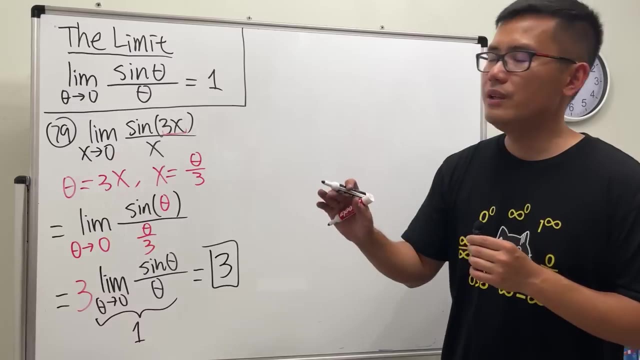 here we just have sine theta over theta and, ladies and gentlemen, this is just equal to one. why, thankfully, we have this secret weapon to use. so it's just one. so we have three times one, and the answer to that is just three, and then we are done. yeah, much better. please do not use. 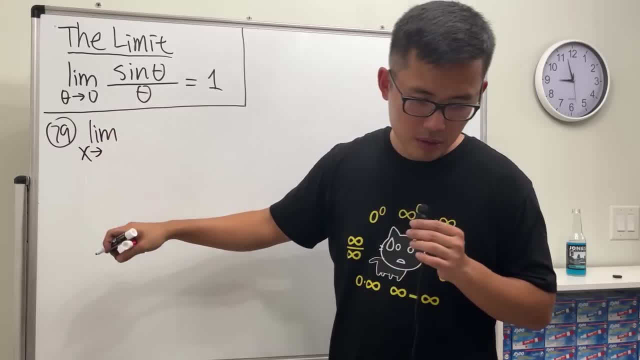 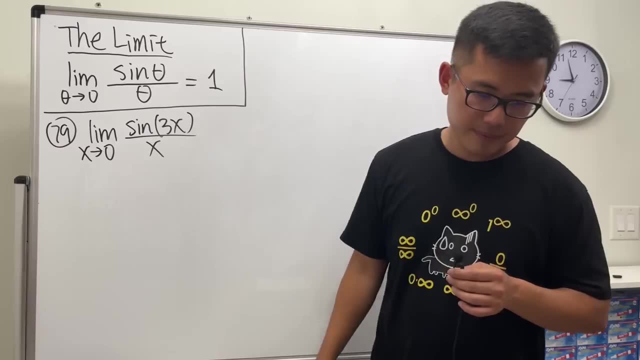 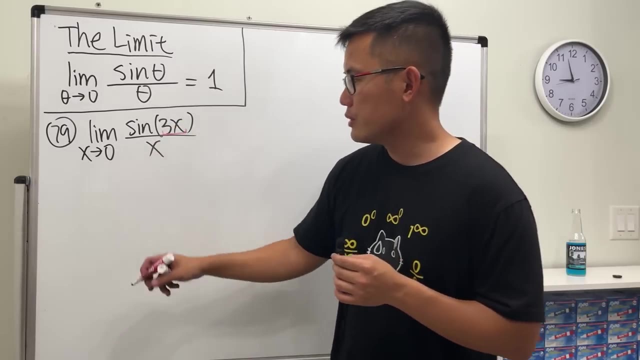 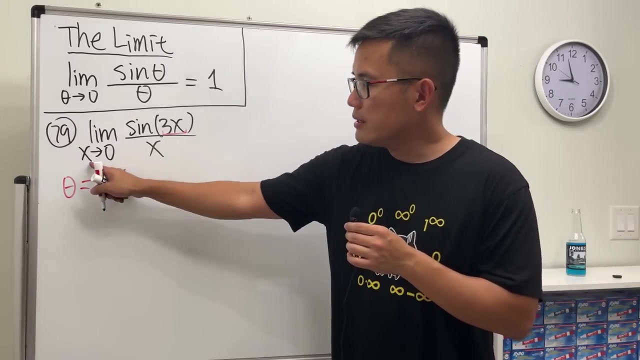 limit as x approaching zero. and then we have sine of 3x over x. okay, here the input is 3x. what we can do is just do a nice substitution, call theta to be 3x and you see, when x is approaching zero, you can put it here: theta is approaching zero as well. good, 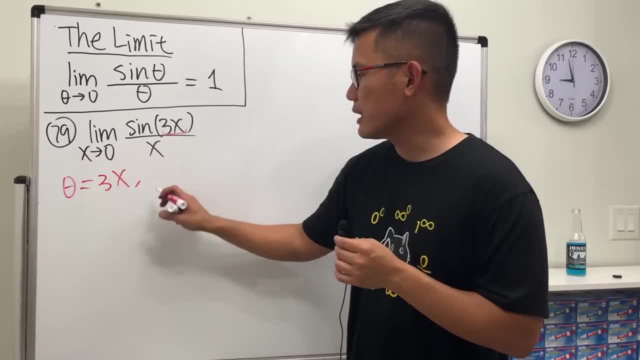 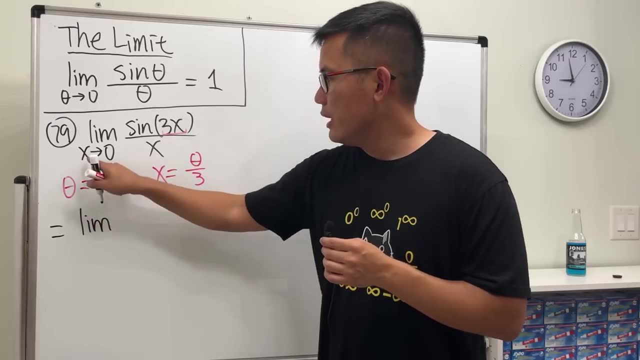 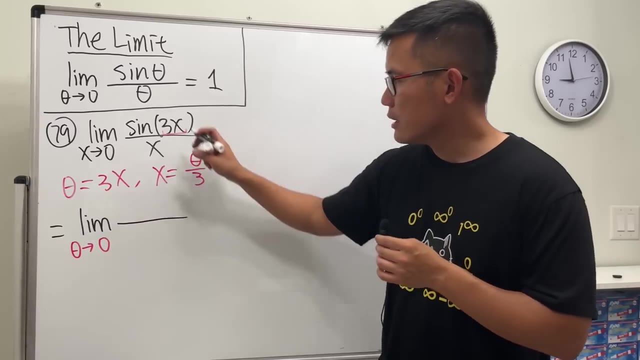 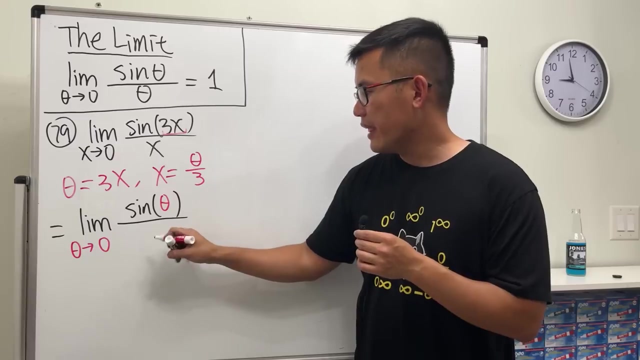 and perhaps we can also solve for x. we can divide the 3 on both sides. this means x is equal to theta over 3.. so you can see, this is going to be the limit. x approaching 0 implies theta will go to 0, and then here we have sine. and then this right here is theta inside now, and then the x is theta. 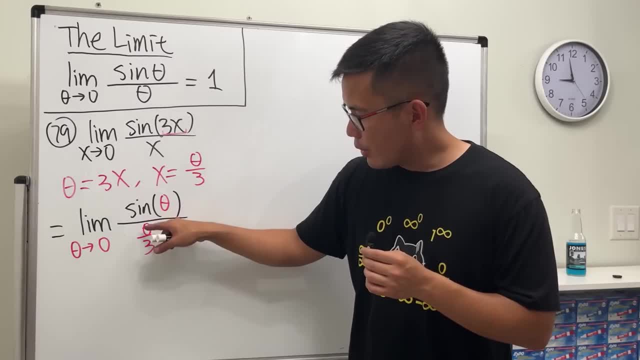 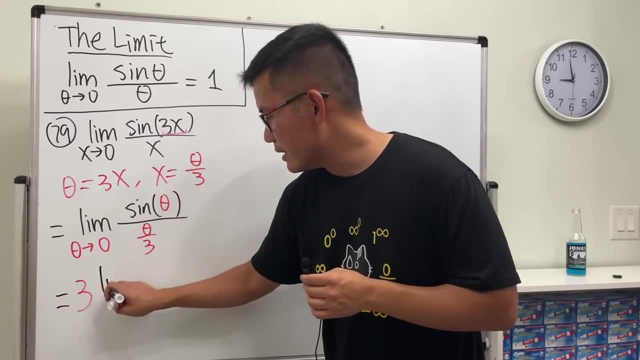 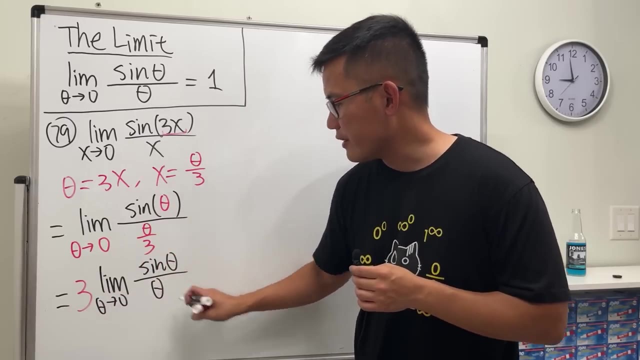 over 3.. but you know the over 3 in the denominator we can put it up right here. so all in all we can say this right: here is 3 times the limit as theta going to 0, and then here we just have sine theta over theta. 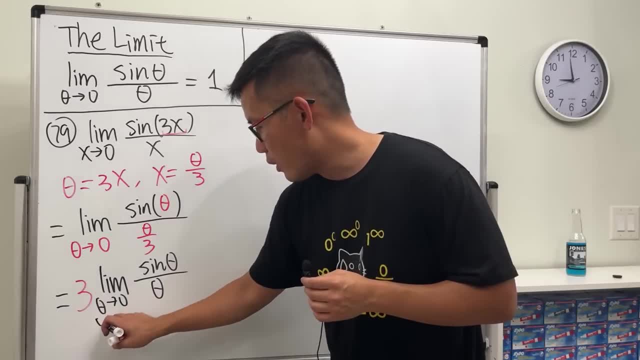 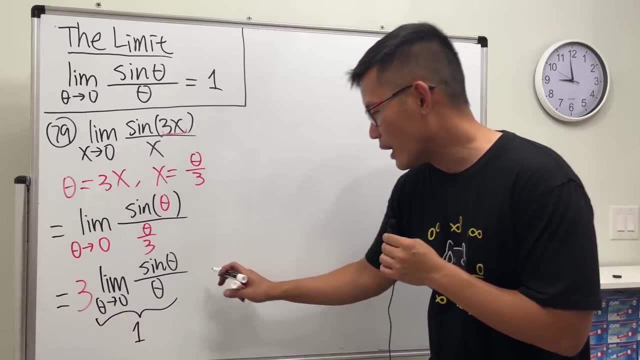 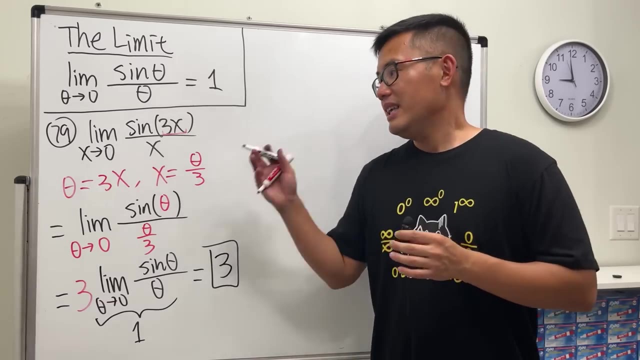 and, ladies and gentlemen, this is just equal to 1.. why, thankfully, we have this secret weapon to use. so it's just one. so we have three times one, and the answer to that is just three, and then we are done. yeah, much better. please do not use lapito's rule for this one. seriously, just use the. 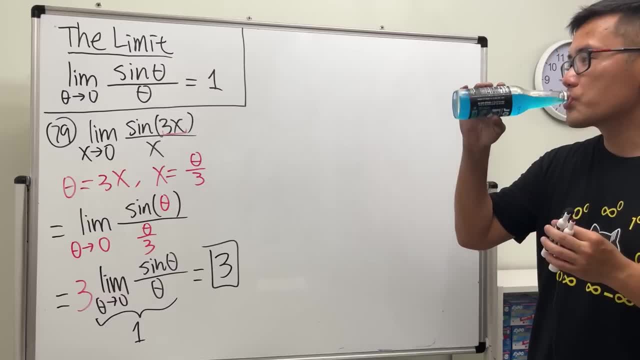 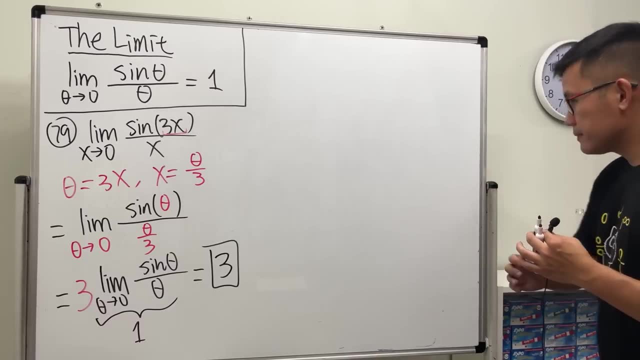 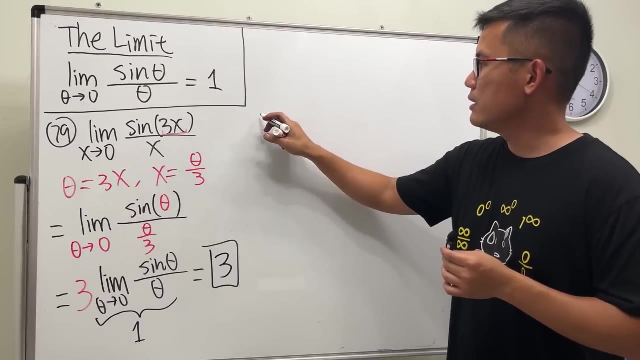 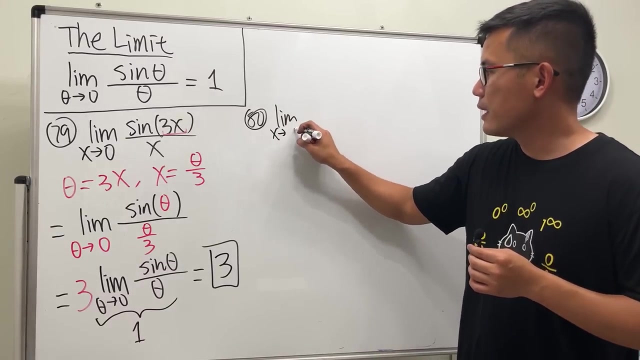 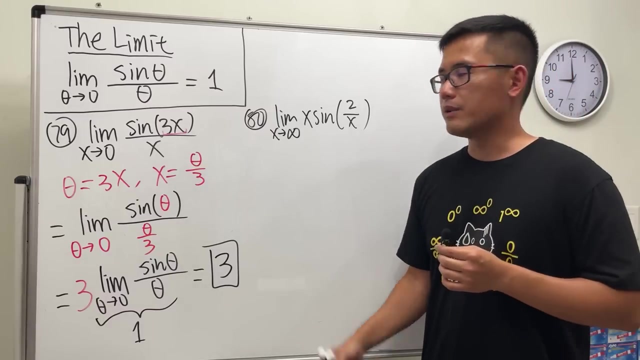 limit. all right, much better this way. much better, this way, all right. hey, let me put it down right here. okay, another one limit as x approaching infinity, and here we have x times sine of 2 over x. wow, this is infinity situation. same thing we can do, it, don't worry. 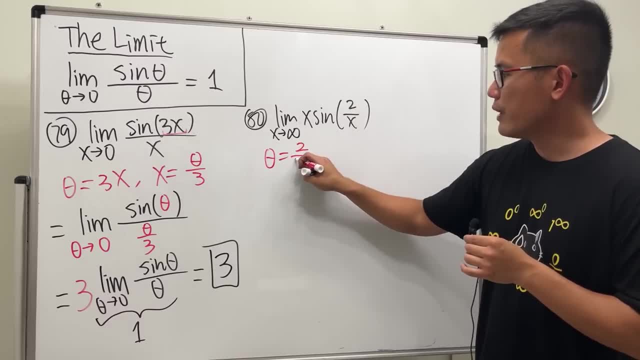 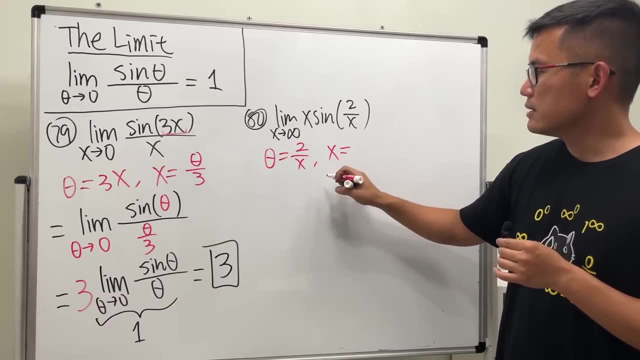 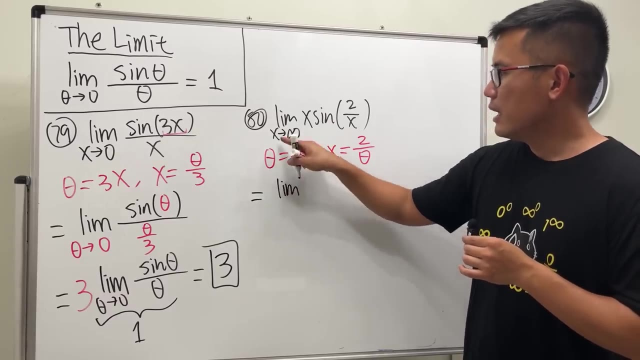 let's call theta to be the input, which is 2 over x. perhaps that's so for x? yeah, so multiply x on both sides, divide theta on both sides. this means x is equal to 2 over theta. check this out. here we have the limit when x is approaching infinity. put it here: 2 over infinity is 0. 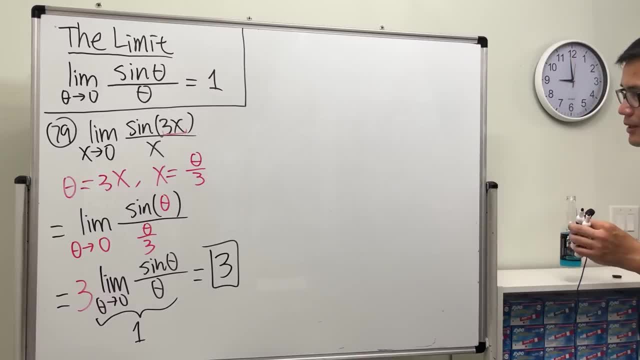 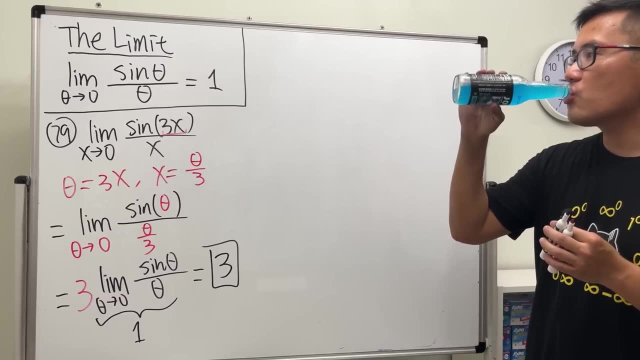 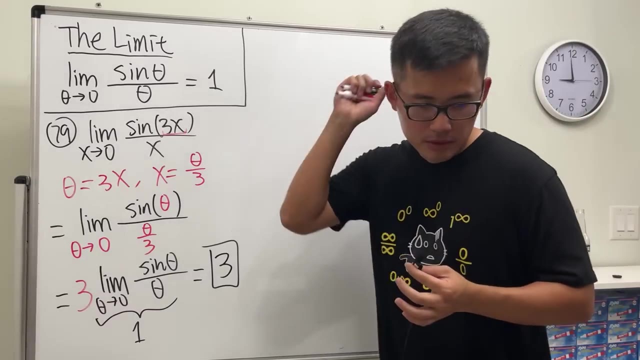 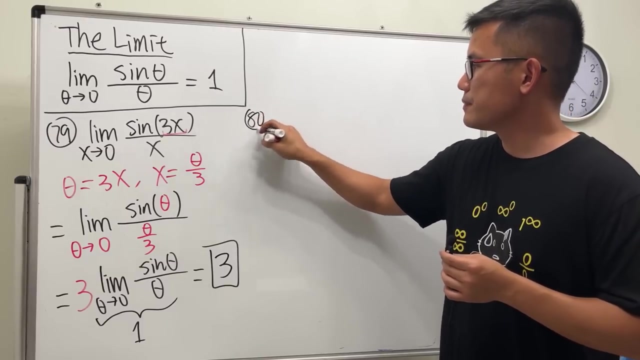 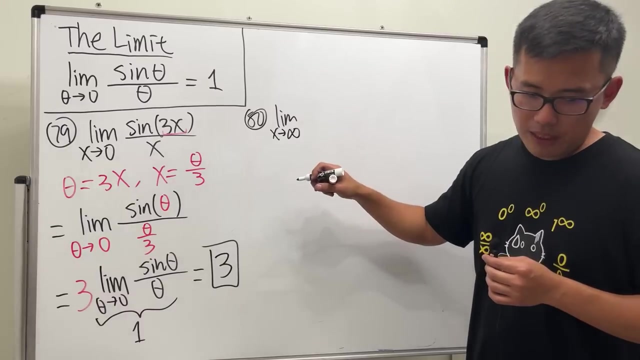 lapito's rule for this one, seriously, just use the limit. all right, much better this way, much better, this way, all right, and let me put it down right here. okay, another one limit as x approaching infinity, and here we have x times sine of 2 over x. 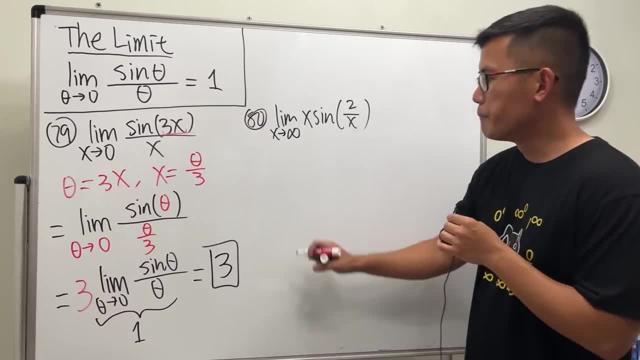 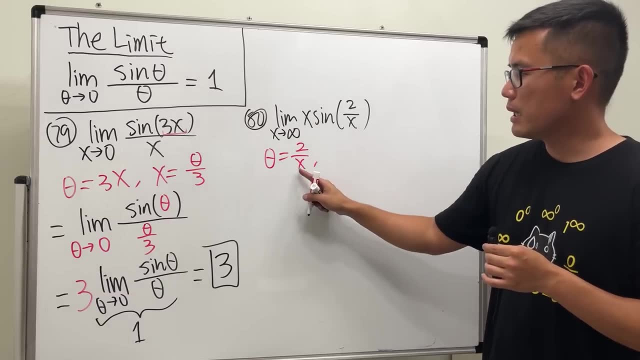 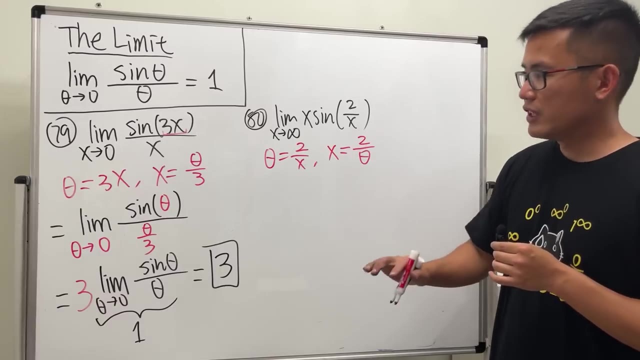 wow, this is infinity situation. same thing. we can do it, don't worry. let's call theta to be the input, which is 2 over x. perhaps that's so for x? yeah, so multiply x on both sides, divide theta on both sides. this means x is equal to 2 over theta. check this out: here we have the limit when x is. 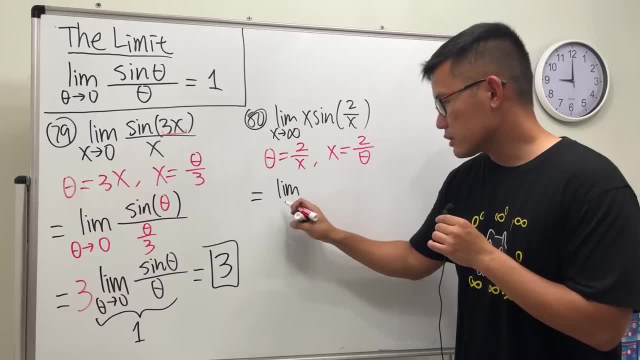 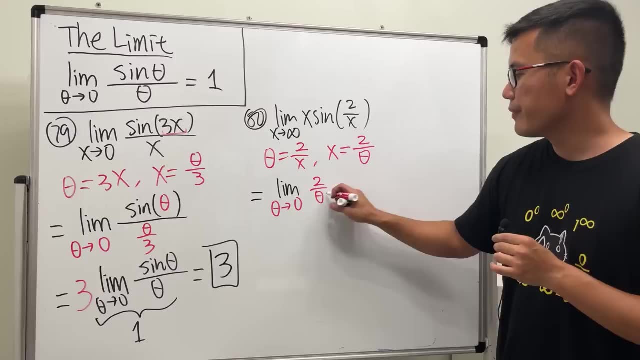 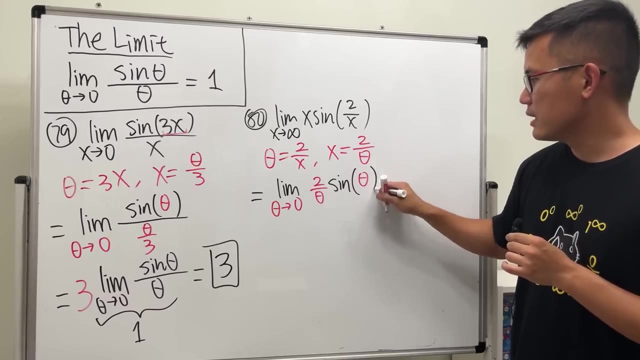 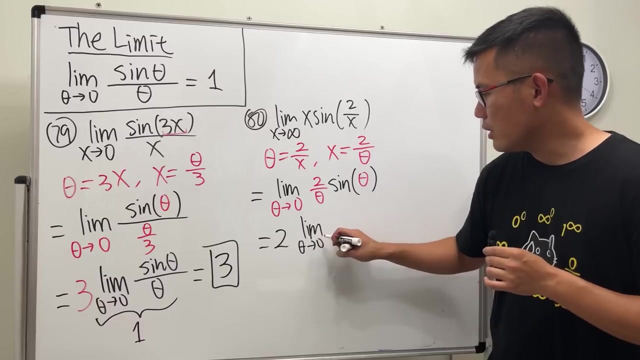 approaching infinity. put it here: 2 over infinity is 0, so theta is approaching 0. good, what's x? that's 2 over theta. and then we have sine and the input is 2 over x, which is theta. great 2 can be brought to the front, yes. and then we have the limit, and then theta approaching 0, and then what's this? 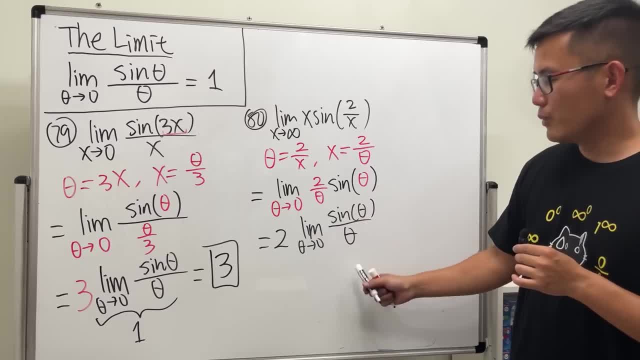 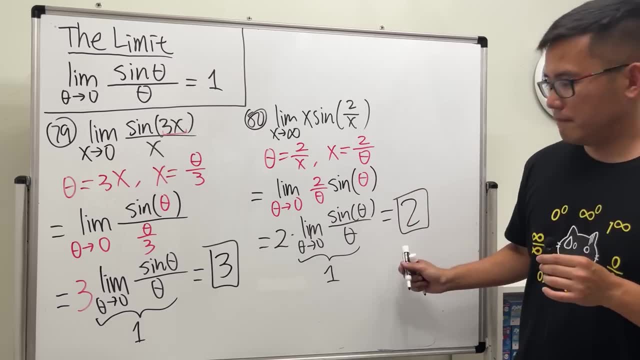 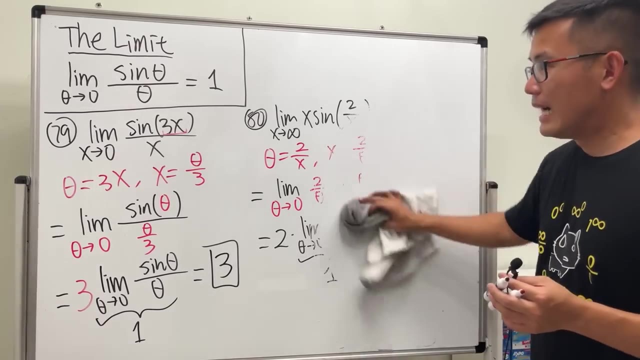 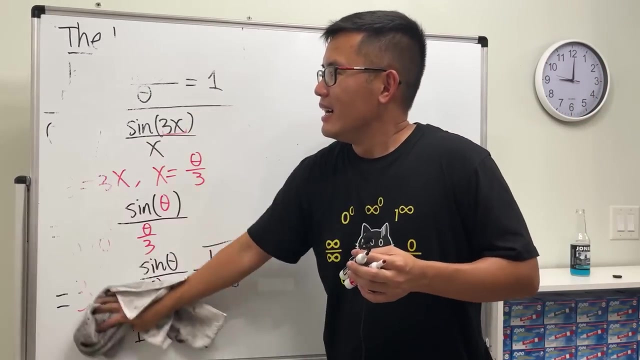 what's this sine theta, over theta, which is 1 oh no, 2 times 1, 2 done, all right. am i happy that the secret weapon isn't over? no, am i happy now? what's coming next? not really, but i don't know why i put a hardest part at the end when my energy level is the lowest. 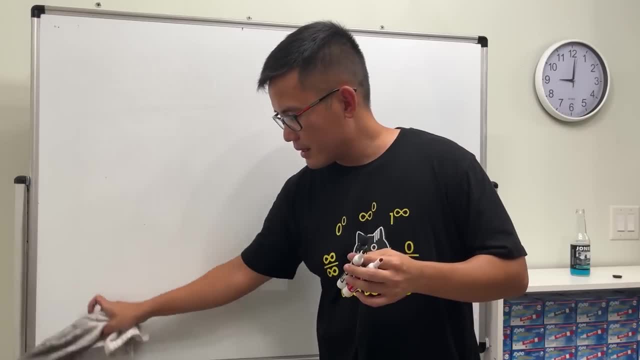 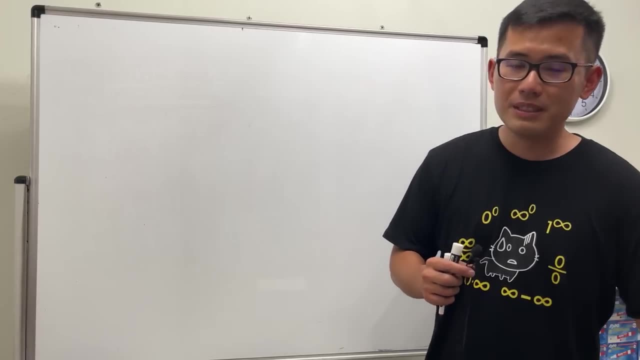 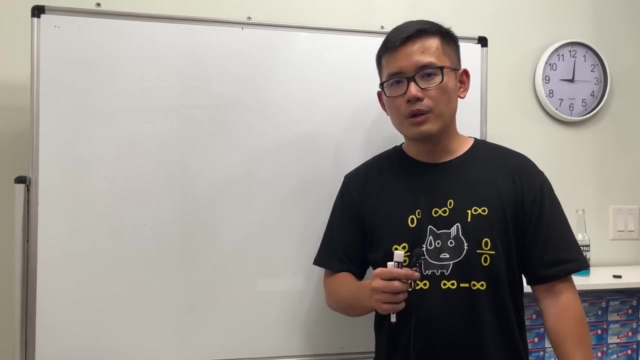 but let's see we can handle it, no worry. so by now i will say, uh, this should cover enough of your calc 1, cal 2 limits. and then, uh, for epsilon delta definitions depends if your teacher, your professor, goes over it or not. if you are at the unit, if you're at a four-year university, then most likely. 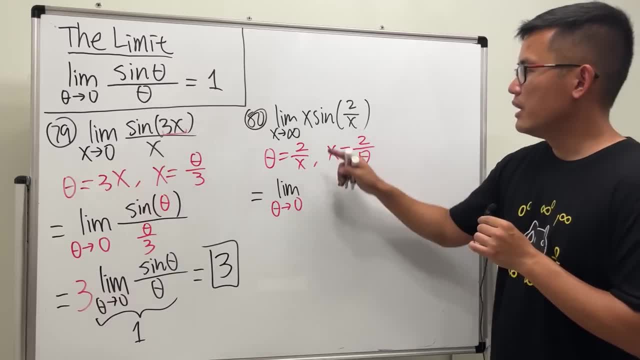 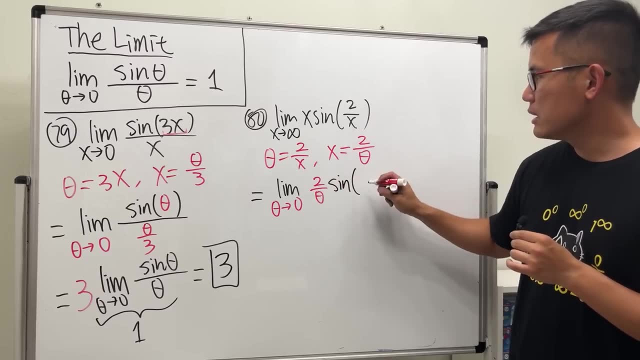 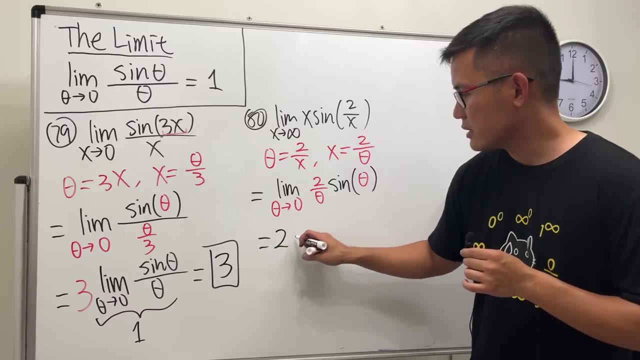 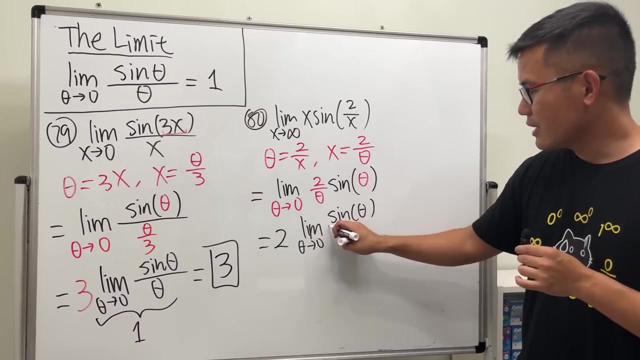 so theta is approaching 0. good, what's x? that's 2 over theta. and then we have sine, and the input is 2 over x, which is theta. great 2 can be brought it to the front, yes. and then we have the limit, and then theta approaching zero. and then what's this? what's this sine? theta over theta, which is. 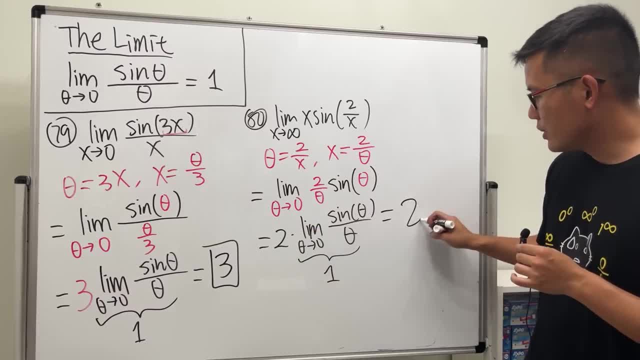 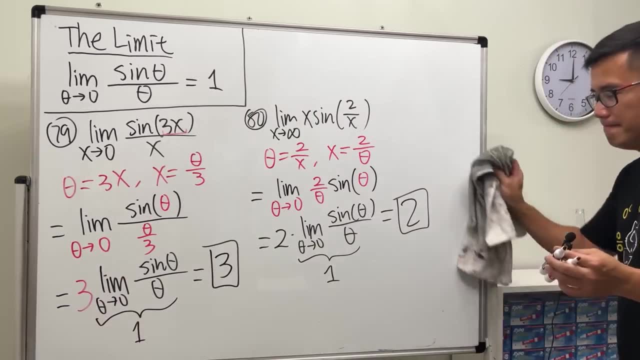 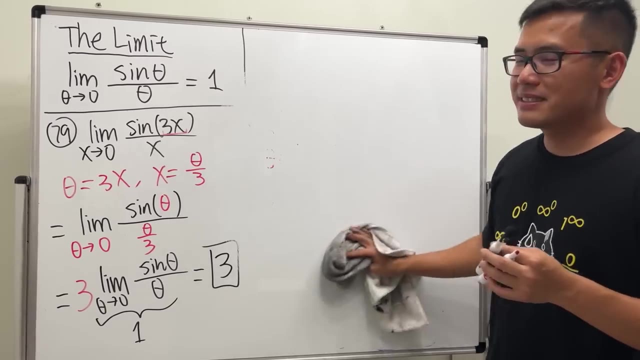 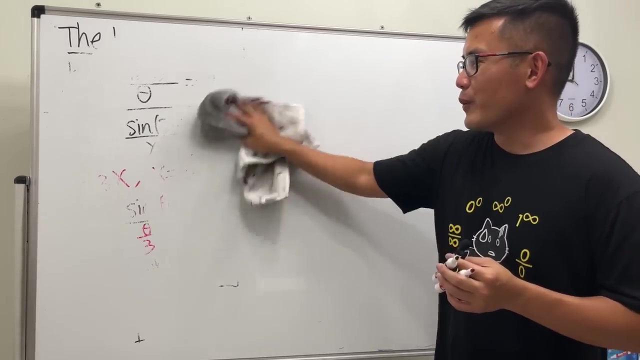 one, oh no, two times one. two done, all right. am i happy that the secret weapon isn't over? no, am i happy now? what's coming next? not really, but i don't know why i put a hardest part at the end when my energy level is the lowest. 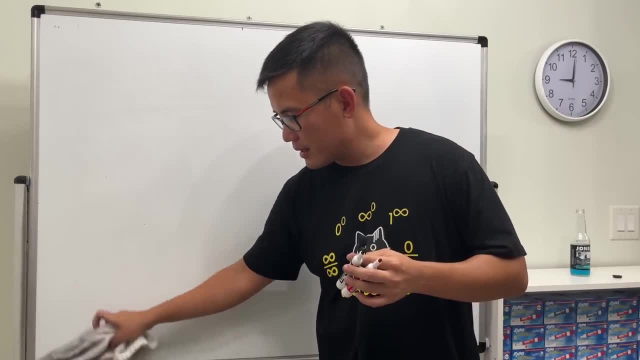 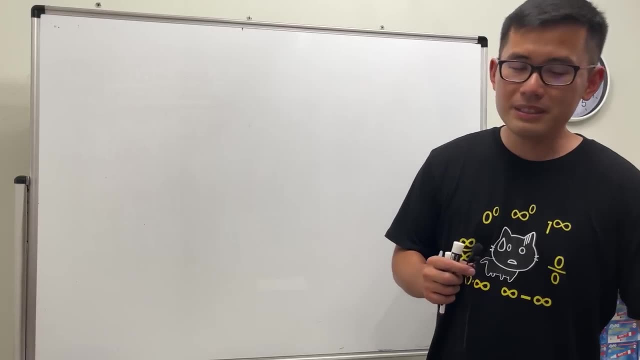 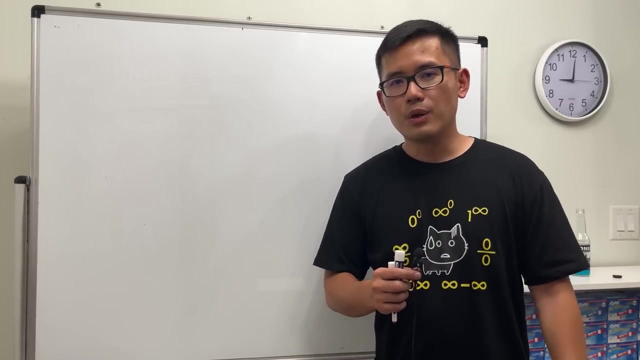 but let's see we can handle it, no worry. so by now i will say, uh, this should cover enough of your call one, call two limits. and then, uh, for epsilon delta definitions depends if your teacher, your professor, goes over it or not. if you are at the unit, if you're at a four-year university, then most likely you will have to know. 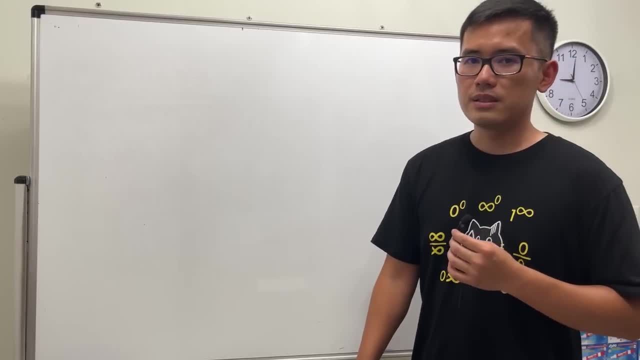 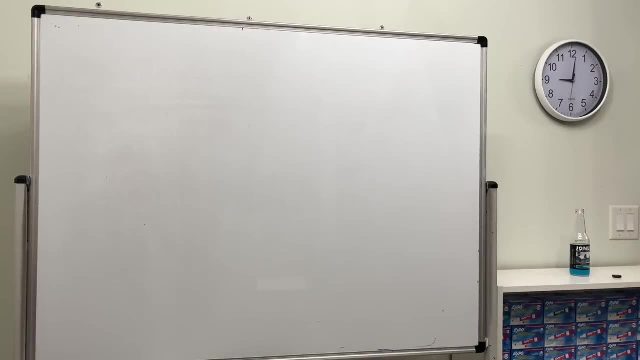 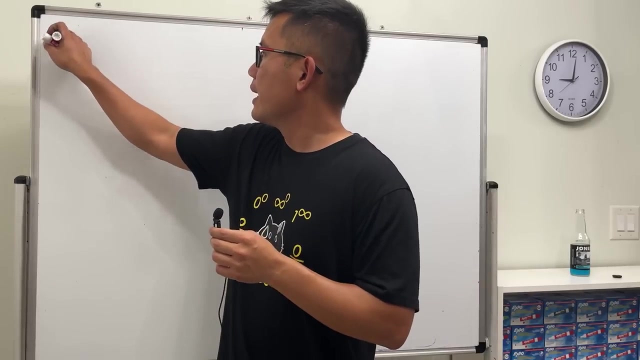 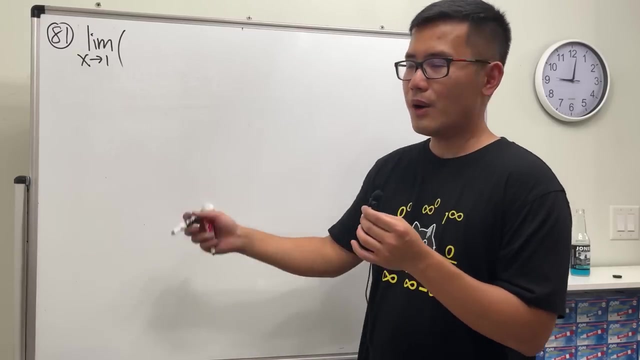 how to do the epsilon delta definition. but don't worry, i'll show you guys four words on how you can keep track and then organize everything. five hours and 26 minutes, all right. so here is number 81. we have the limit as x approaching one. you are going to be like wow. 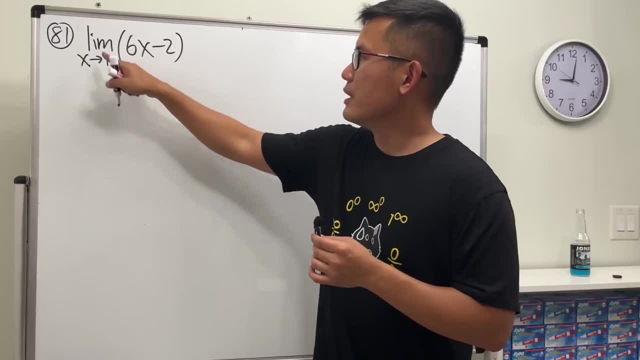 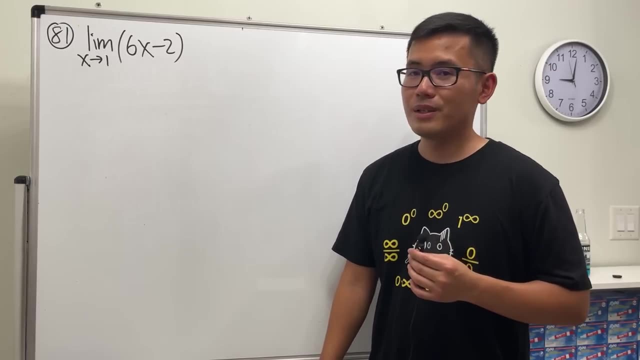 seriously, this is the question. yes, this is the question. x approaching 1 and we have 6x minus 2.. that's number 81.. so easy, right? yes, we can just put a 1 in here. i'll show you guys the work if. 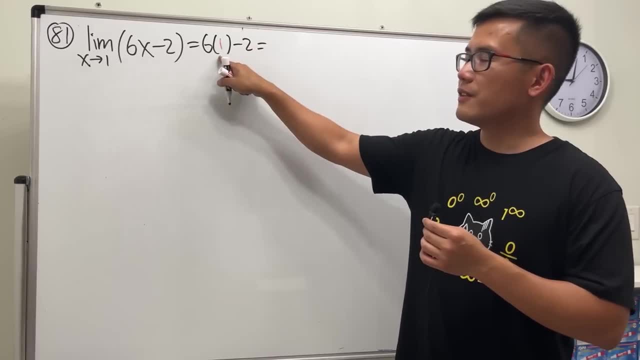 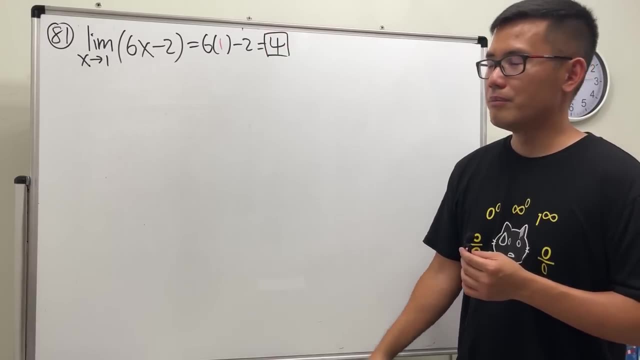 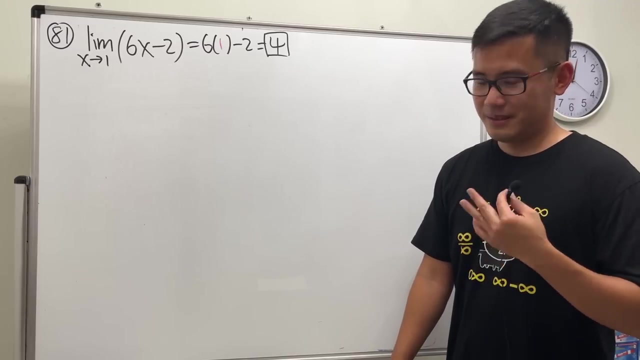 you would like 6 times 1 minus 2, that's 6 minus 2 is 4.. hey, we are done. yay, but how do we know that this is the answer is actually true? yes, we will have to prove it. how, though? just like what i mentioned earlier? 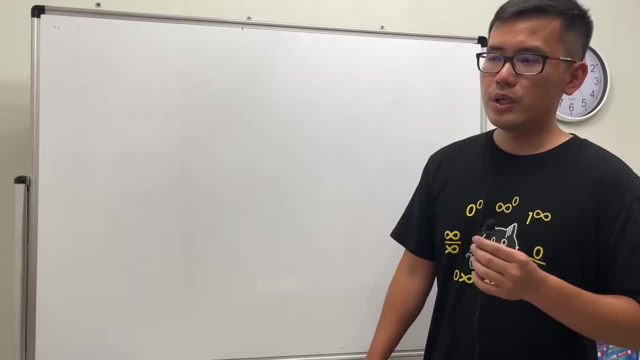 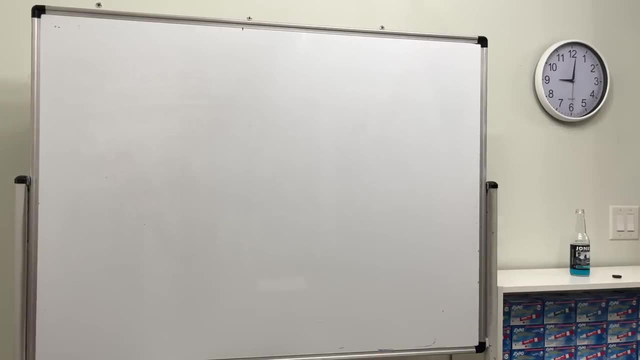 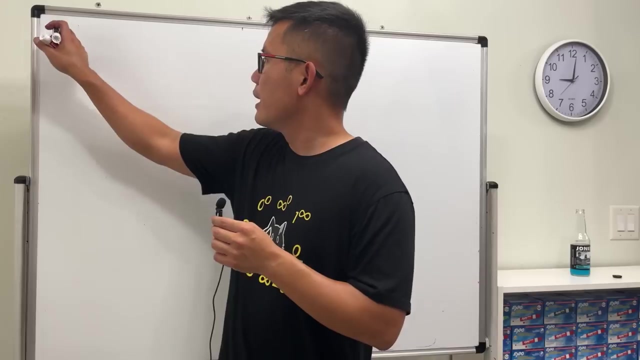 you will have to know how to do the epsilon delta definition. but don't worry, i'll show you guys four words on how you can keep track and then organize everything. five hours and 26 minutes, all right. so here is number 81. we have the limit as x approaching one. 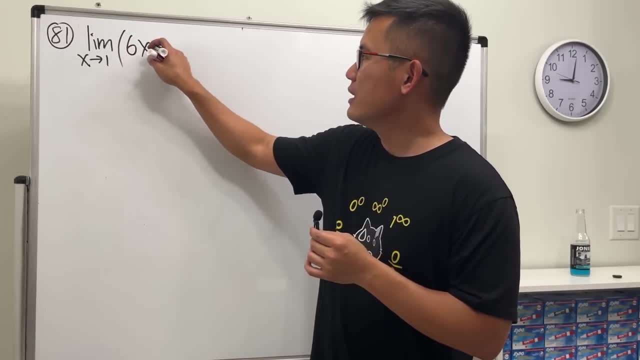 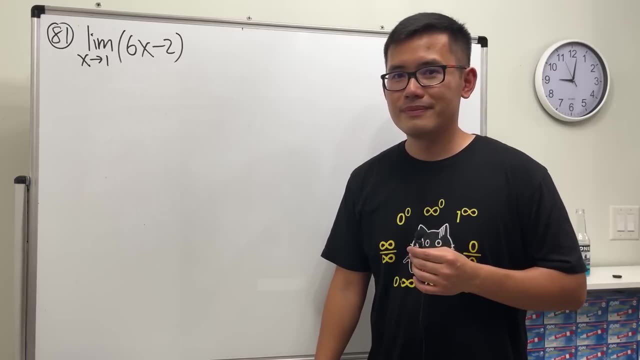 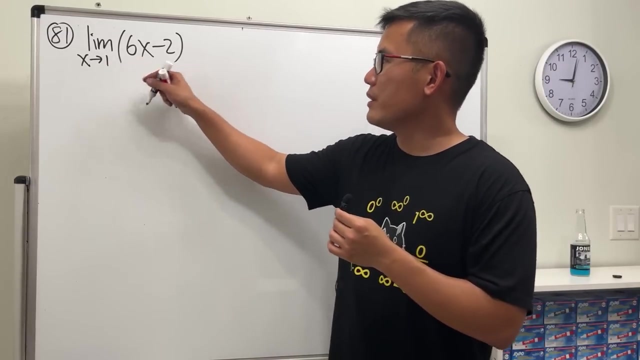 you are going to be like: wow, seriously, this is the question. yes, this is the question. x, approaching 1, and we have 6x minus 2.. that's number 81. that's so easy, right? yes, we can just put a 1 here. i'll show you, guys the. 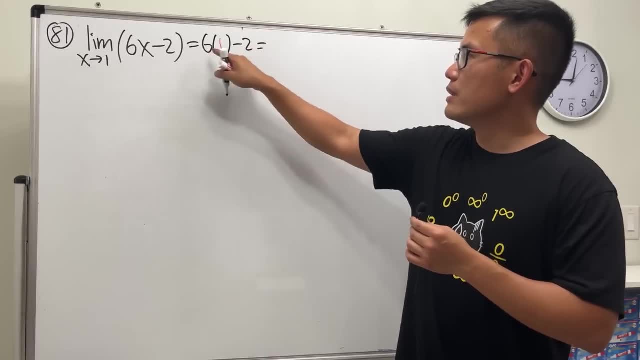 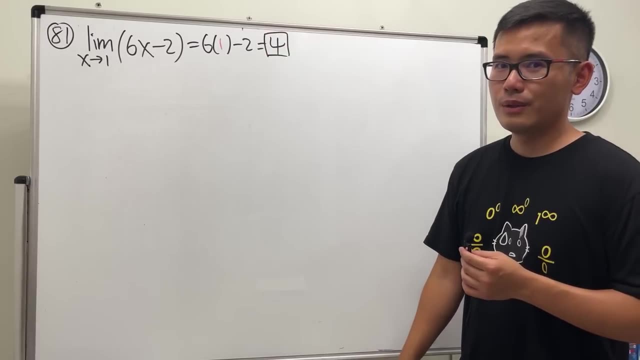 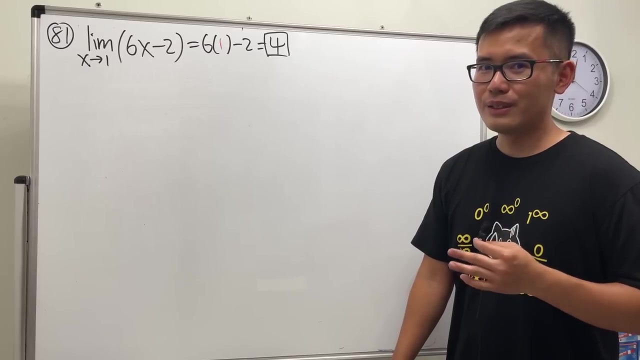 work, if you would like. 6 times 1 minus 2, that's 6 minus 2 is 4.. hey, we are done. yay, but how do we know that this is actually true? yes, we will have to prove it. how, though? just like what i 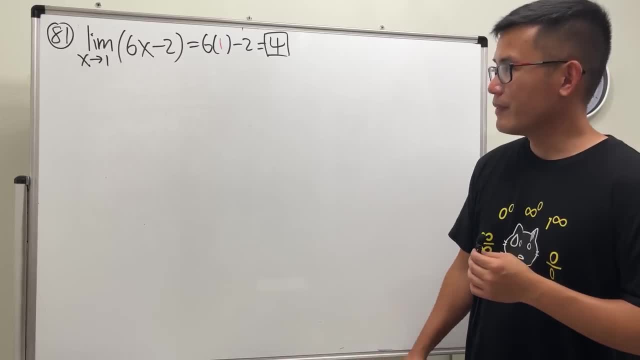 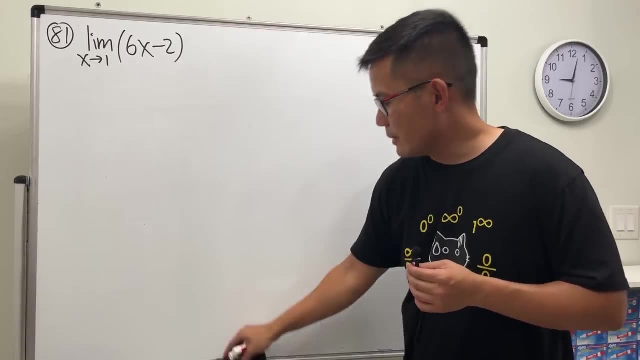 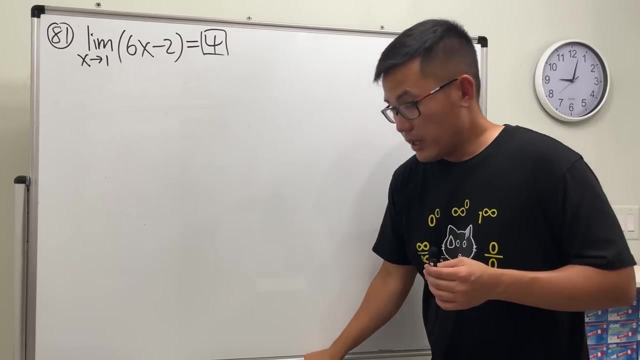 mentioned earlier the epsilon delta definition. I will remind you guys on the side and really depends you have done it or not. Alright, so I'm going to actually Give myself more space. I'm going to put down this right: here is war. Okay, here's the deal. if we have the limit as X approaching some number a, 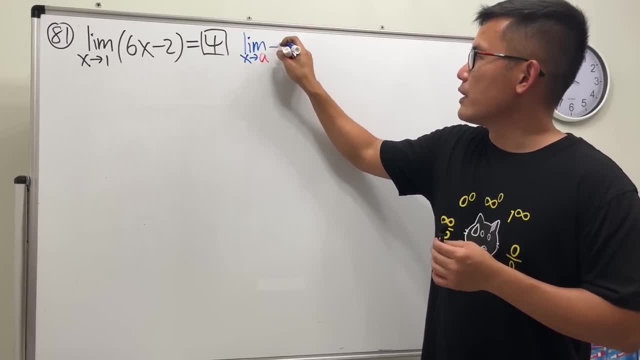 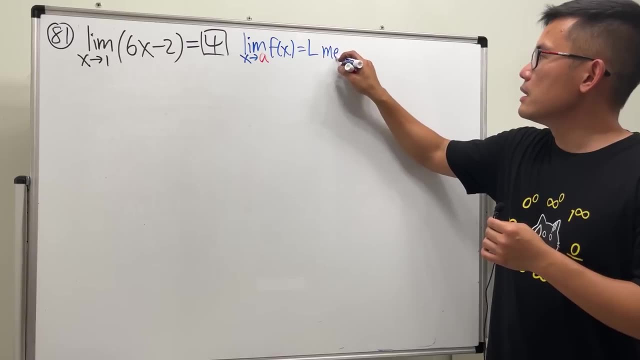 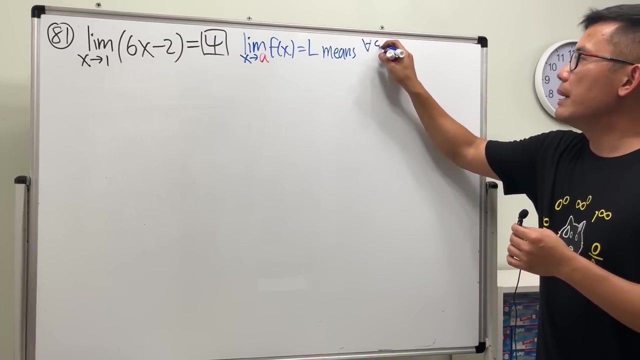 Of some function f of X. if we do end up with some limits, that's going to be out. this right here means You ready? It's mean, I know, but it means for all Epsilon greater than 0, there exists a Delta greater than 0 such that 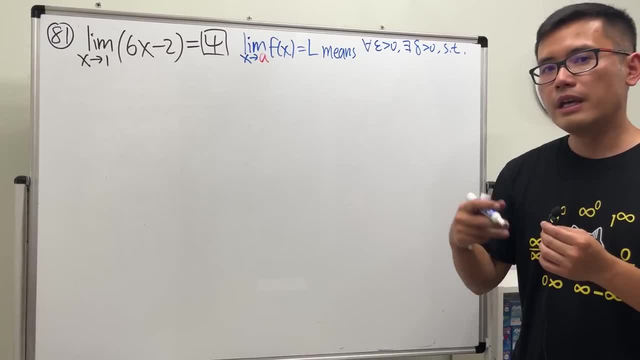 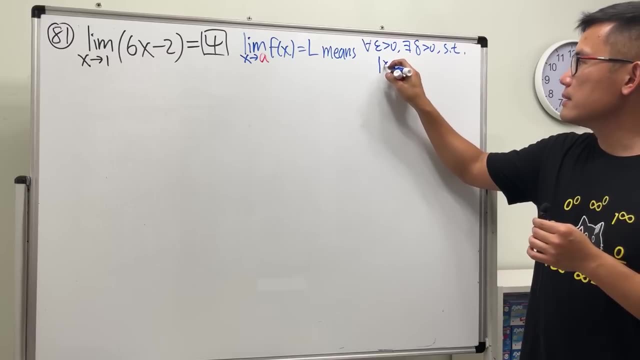 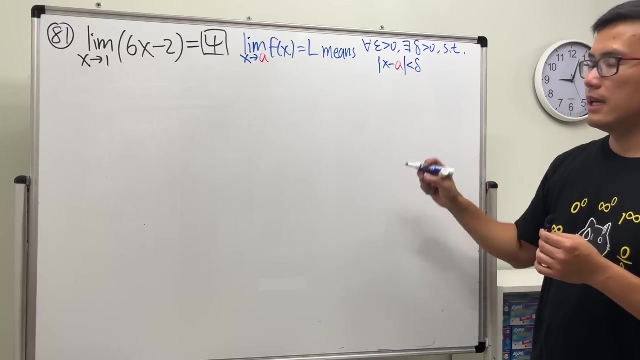 if the distance between X and a is small enough, and for distance means we have the absolute value and it just Track them. So we put absolute value of X minus a. If it's small enough, how small is? no Less than Delta. Okay, and then we do not need X, We do not want X to be a. so we want to say: 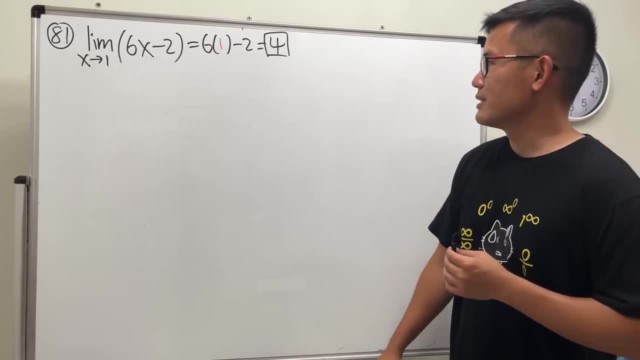 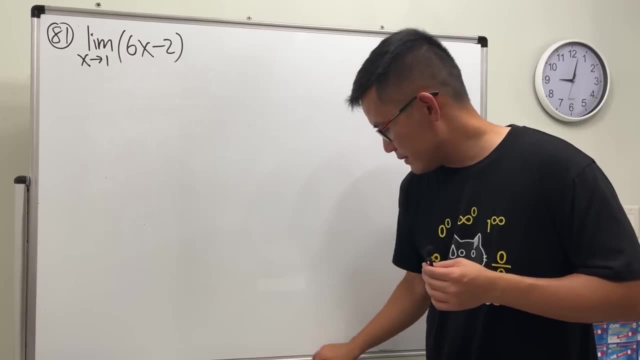 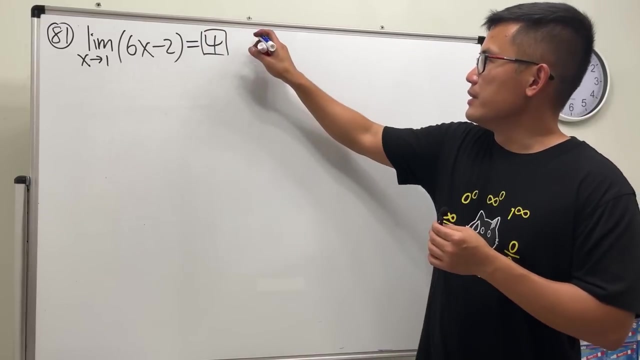 the epsilon delta definition. i will remind you guys on the side and really depends you have done it or not. all right, so i'm going to actually give myself more space. i'm going to put down this right here. it's, or okay, here's the deal. if we have the limit as x approaching some number a, 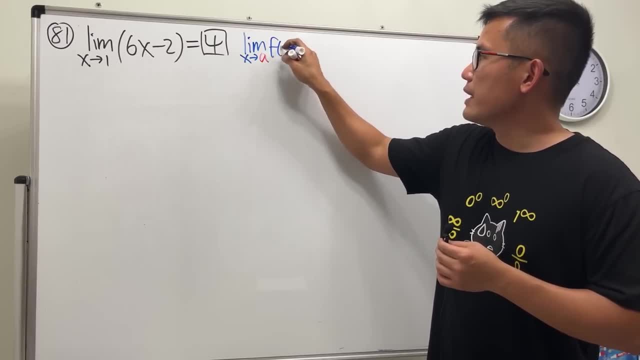 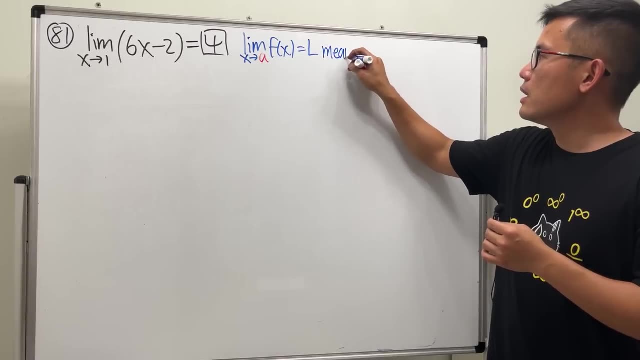 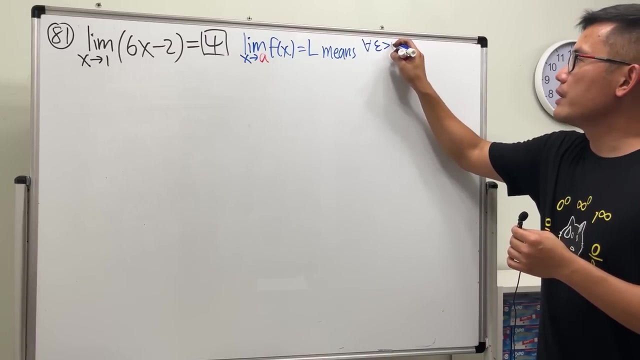 we see. all right, so if we have alphabets, so here's the rule for definition of some function f of x. if we do end up with some limits, that's going to be out. this right here means you're ready. it's mean, i know, but it means for all epsilon greater than zero. 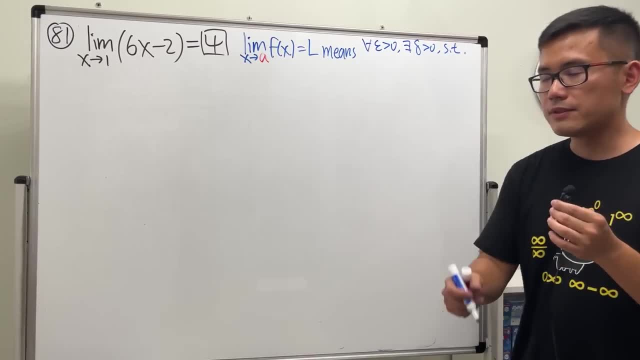 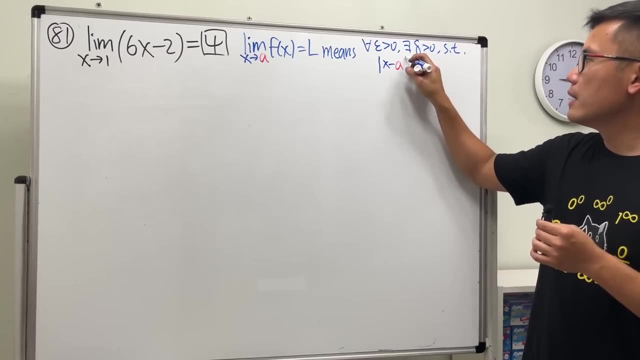 there exist a delta greater than zero, such that if the distance between x and a is more enough- and for distance means we have the absolute value and just subtract five сч from x values them. so we put absolute value of x minus a. if it's small enough, how small is small less than? 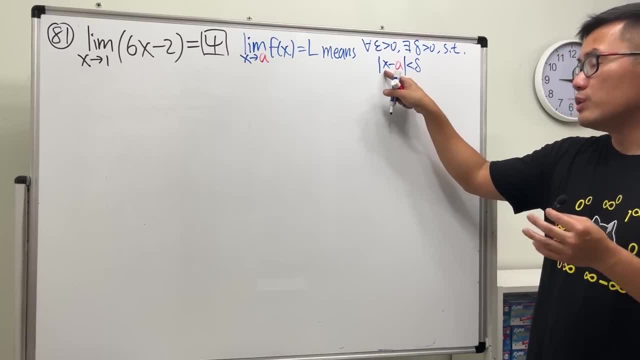 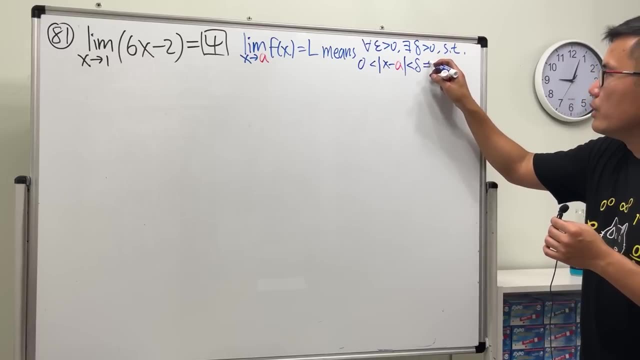 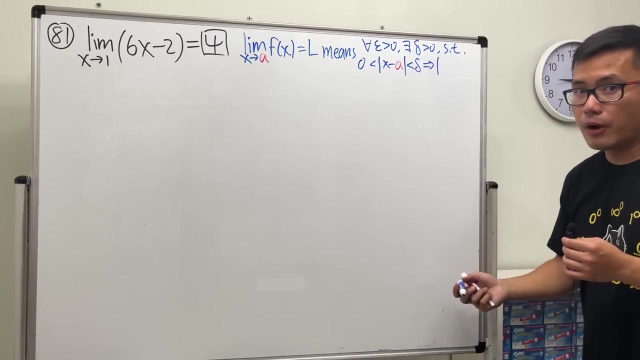 delta. okay, and then we do not need x, we do not want x to be a, so we want to say: this is greater than zero. if this is true, then we must have the absolute value of the. well, it's pretty much the distance between f of x and the limit l. it's small enough as well, but in this case we write: 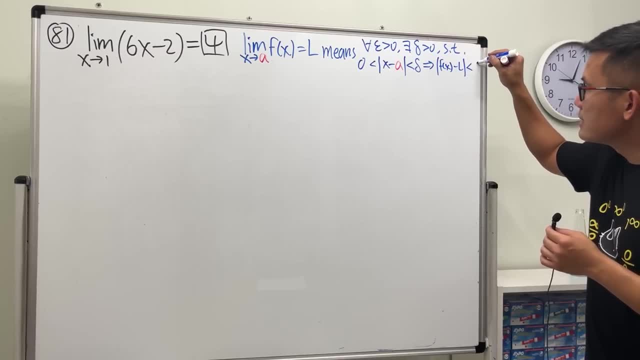 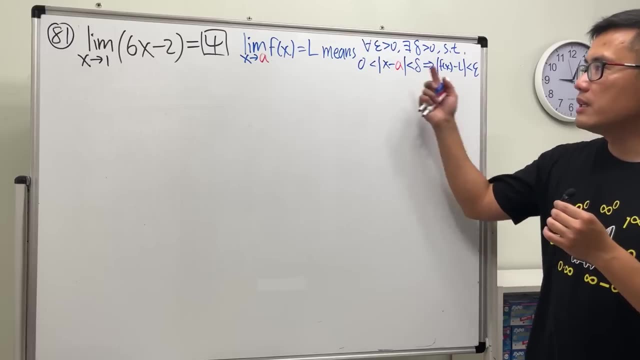 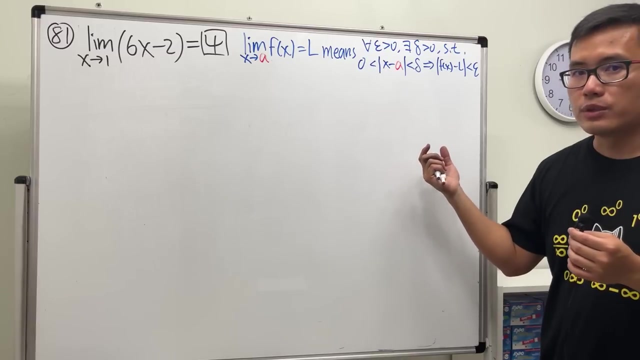 it as f of x minus l to be less than epsilon. yeah, so intuitively it means that you can get as close to l as you would like. then that's. this is just like a formal way to say it, because, again, f of x minus l is the distance between the function and the limit. 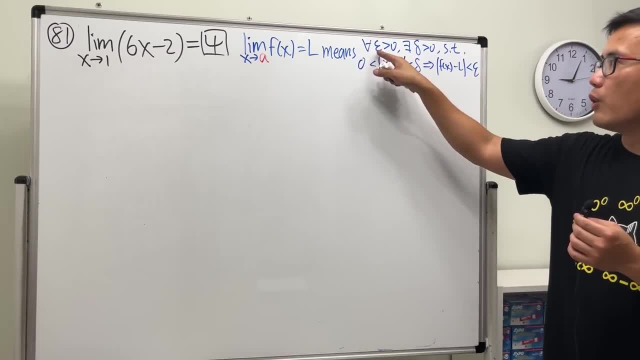 you can make it as close to the limit as you would like. you can make it as small as possible. that's why it's for all epsilon greater than zero and you can make it as small as possible. it's because you can always find a delta greater than zero. so 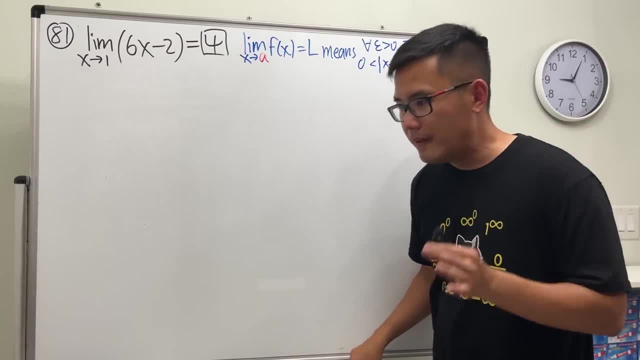 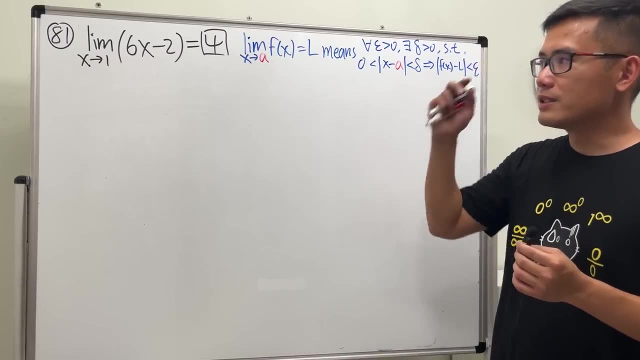 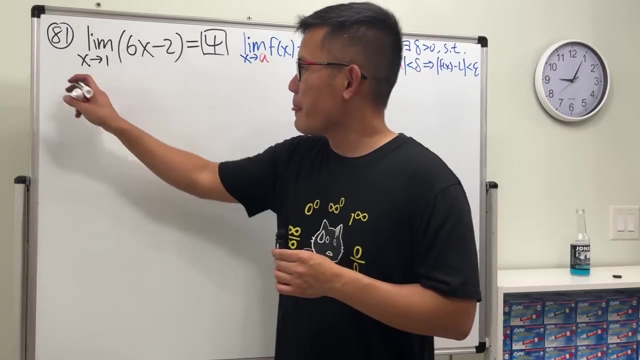 when this happens, this happens. that's the idea. i have a very detailed video going over this, so you should definitely try that, but for now, we will see how to just write the proof. write the proof. write the proof for 10 of them. okay, here we go. how do we write the proof? 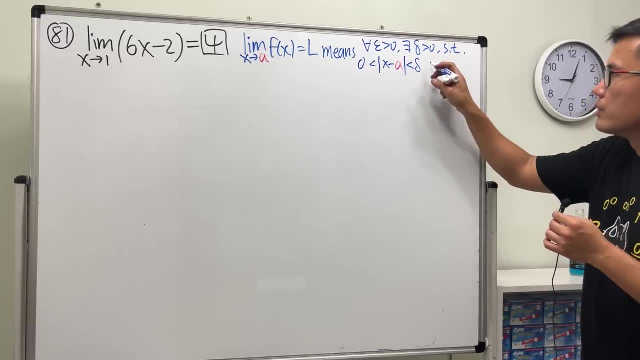 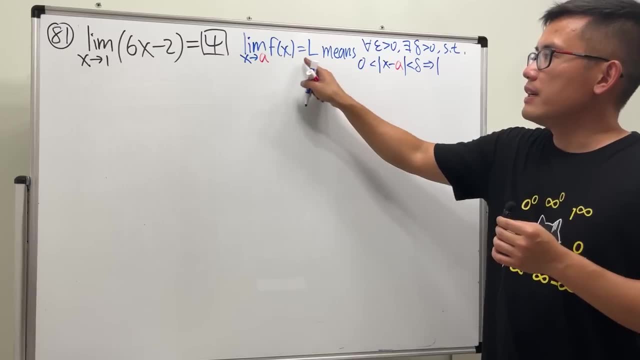 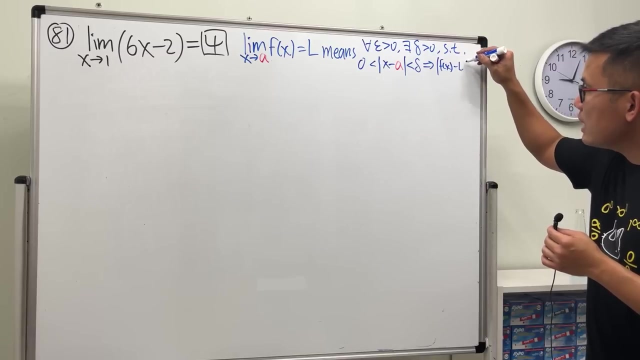 This is greater than 0. if this is true, then we must have the absolute value of the. Well, it's pretty much a distance between f of X and the limit L. It's not enough as well, But in this case we write it as f of X minus L, to be less than epsilon. 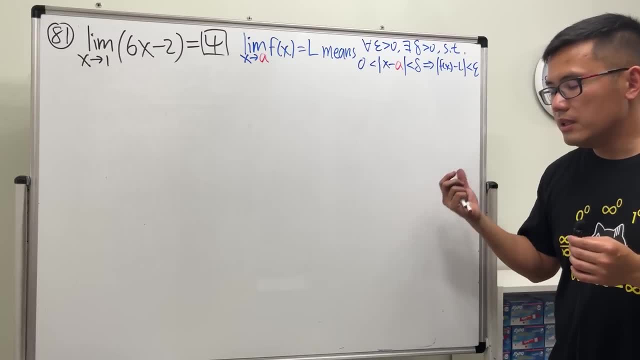 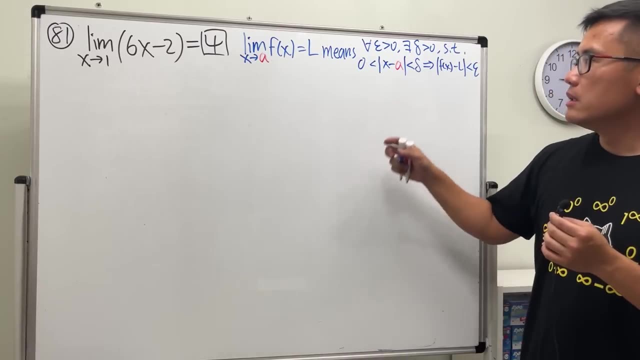 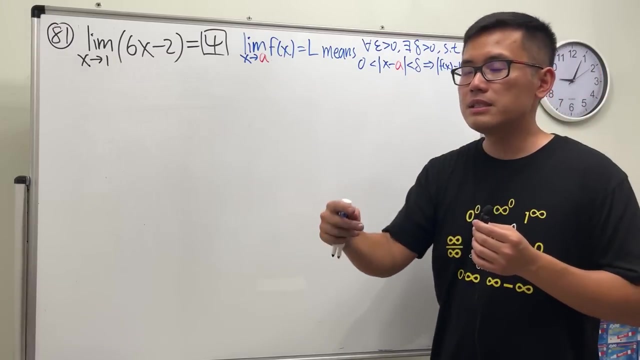 Yeah, so Intuitively it means that you can get as close to L as you would like. Then that's- this is just like a formal way to say it, because again, f of X minus L It's a distance between the function and the limit. you can make it as small as possible. 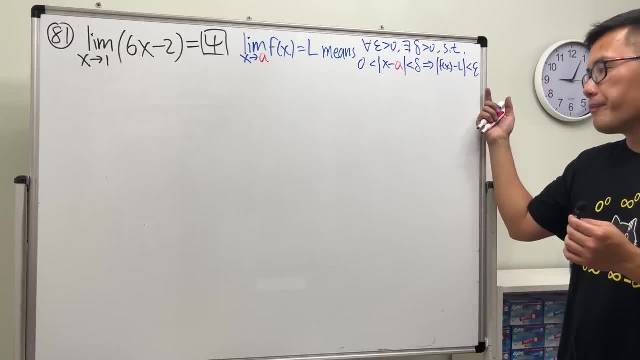 that's why it's for all epsilon greater than 0 and We can make it as small as possible. It's because you can always find a delta greater than 0. So when this happens, this happens. that's the idea. I have a very detailed video going over this. 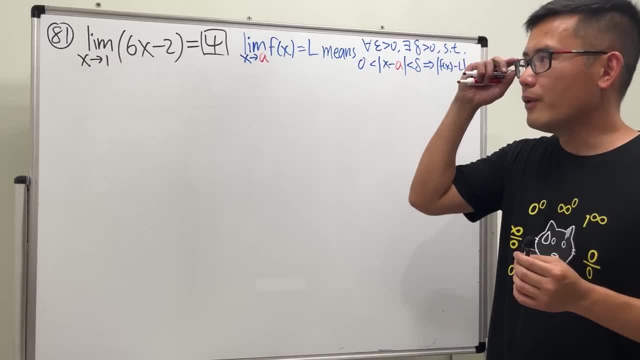 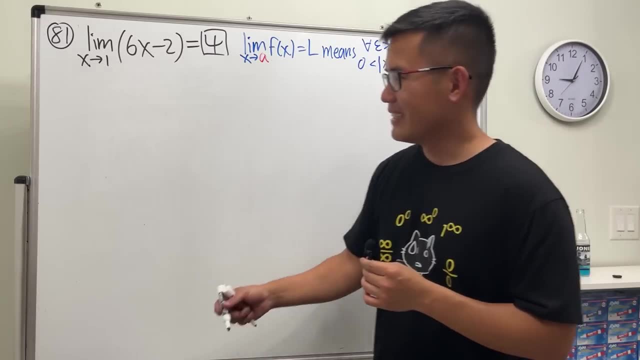 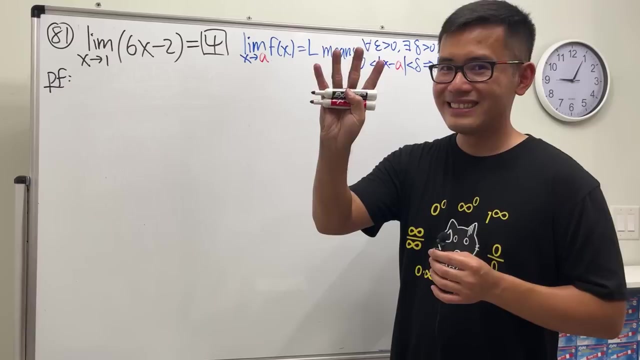 So you should definitely try that, but for now we will see how to just write a proof. write a proof, write a proof for 10 of them. Okay, here we go. how do we write proof? write down P first. everybody will be happy For words, for words, that's going to make everything much, much, much, much much. 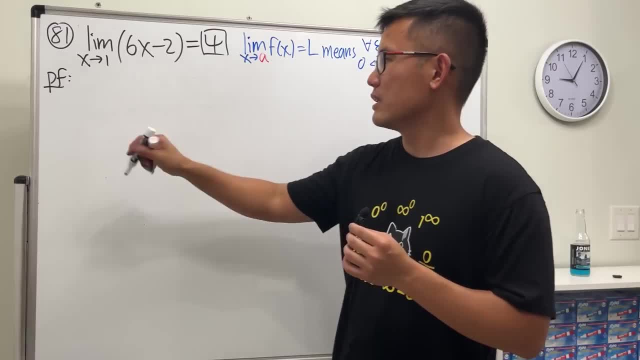 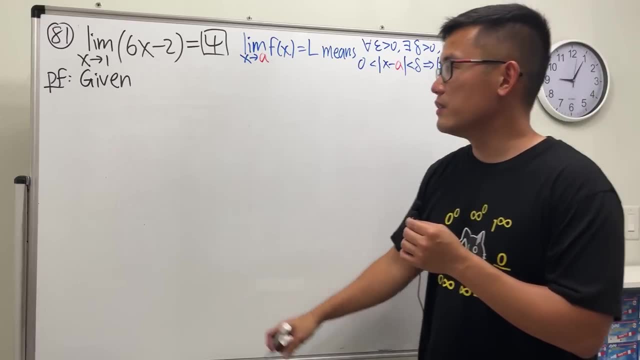 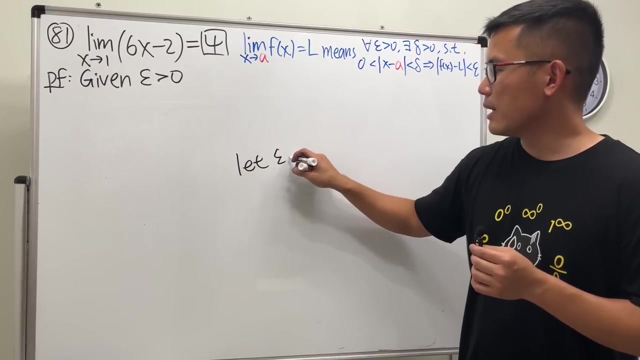 Clear, systematic, easy to follow. first word: given. Why, When you see, for all right, just start with the proof by saying given, and you can just say given Epsilon greater than 0, and some people might say you should say let epsilon Be greater than 0, like this, and then be R. 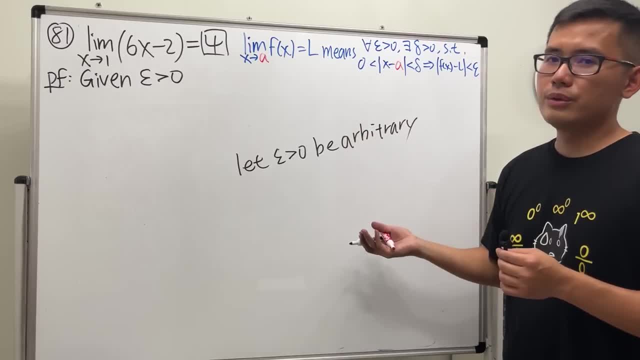 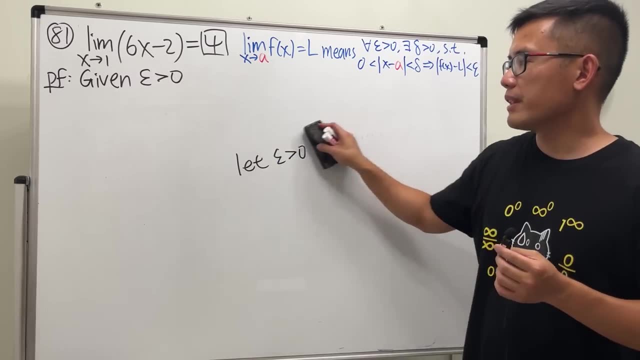 be Cherry, But that's cool too. You know, if you say something like this to some more like a mathematician, and if you will write given Epsilon greater than 0, That's true and concise and the people wouldn't get mad at you. So either way, but given, I think it's okay. 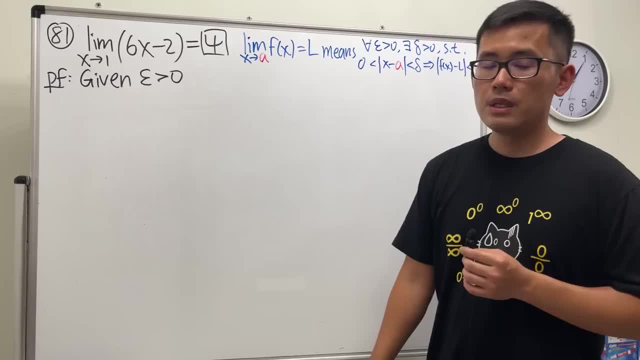 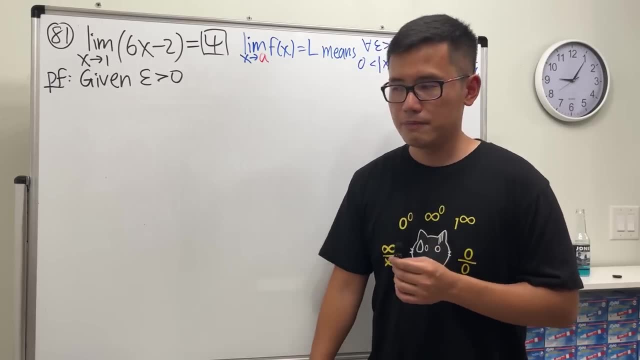 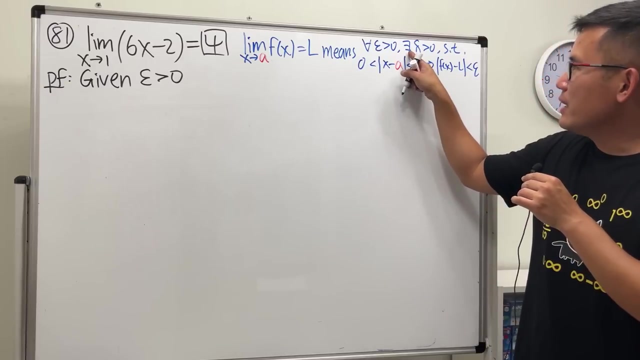 So you always start give an Epsom greater than 0 If I ever ask my students Epsom Delta definition on the test, if you put this down, I'll give you a point Among like 10 points. Anyway, anyway, Next, you see that right here, says there exists. 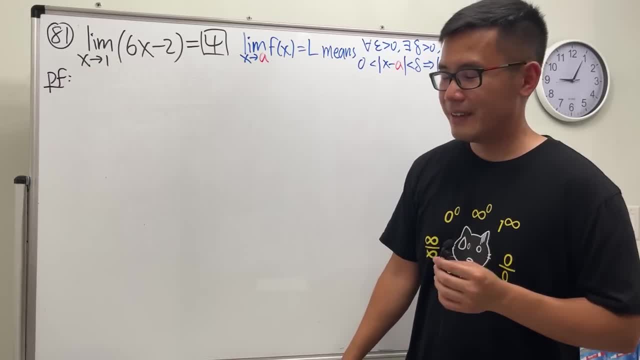 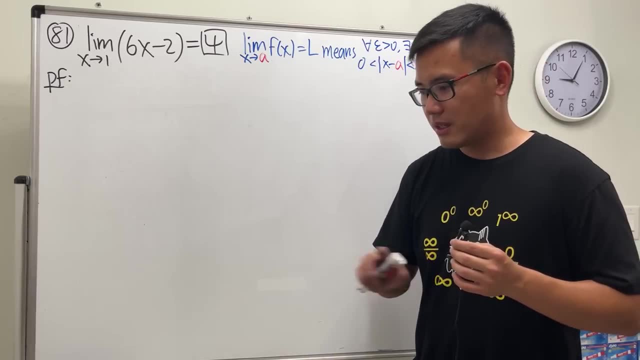 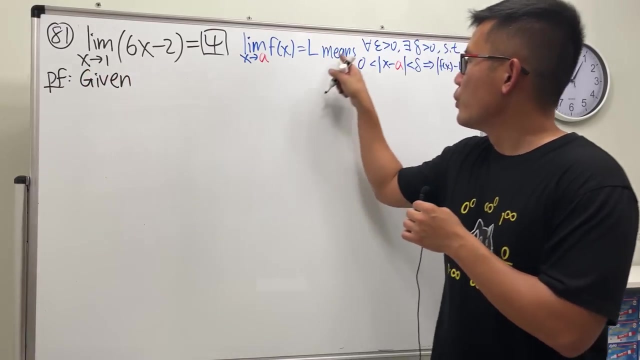 write the proof, write on p first, everybody will be happy. four words, four words, that's going to make everything much, much, much, much much clear, systematic, easy to follow. first word: given why, when you see, for all right, just start with the proof by saying given and you can just say given. 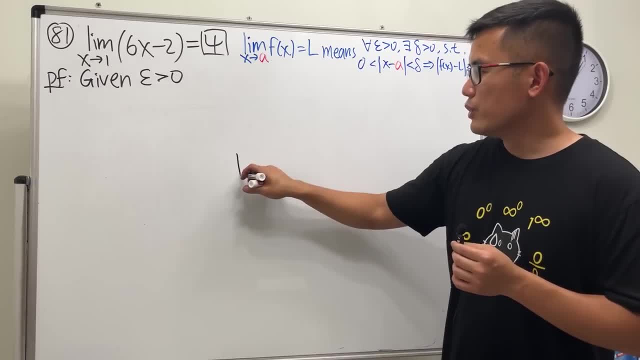 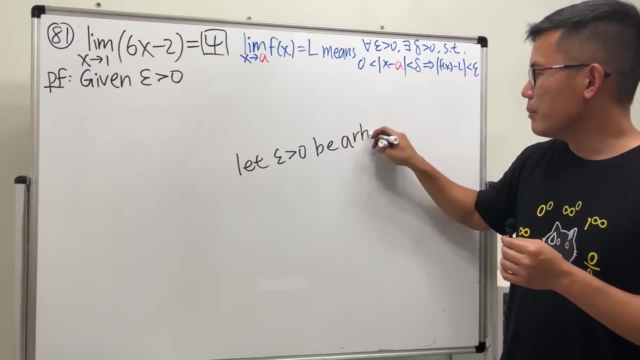 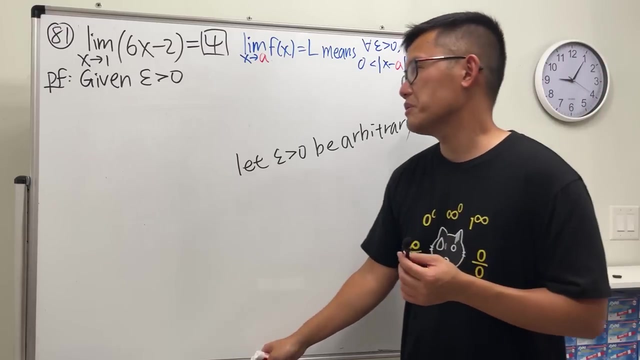 epsilon greater than zero. and some people might say you should say: let epsilon uh be greater than zero, like this, and then b r b cherry. but that's cool too. you know, uh, if you say something like this, you sound more like a mathematician. and if you write, give an epsilon greater than zero, that's true in. 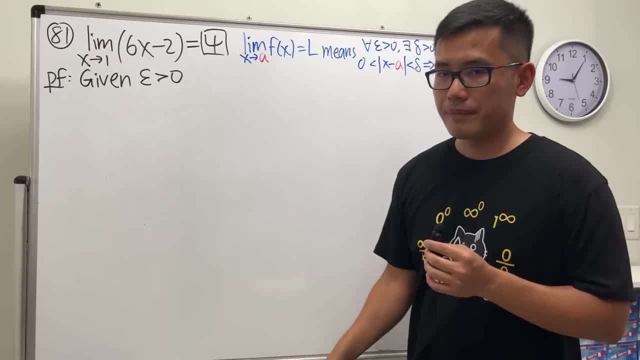 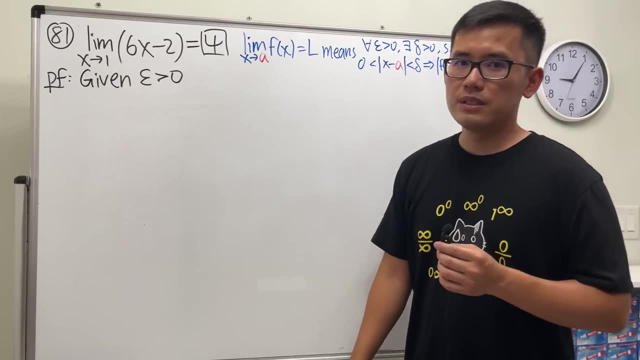 context and the people wouldn't get mad at you. so either way, but given, i think it's okay. so you always start, give an epsilon greater than zero if i ever ask my students: uh, epsilon, delta definition on the test. if you put this down, i'll give you a point. 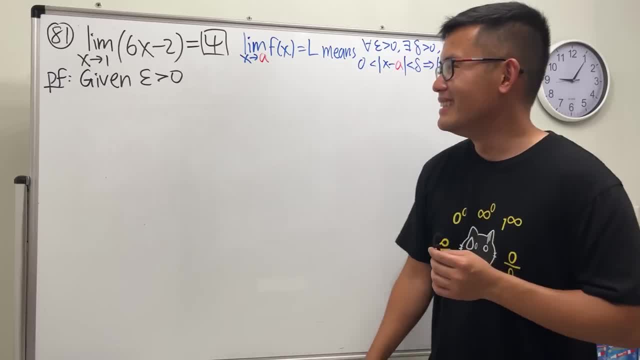 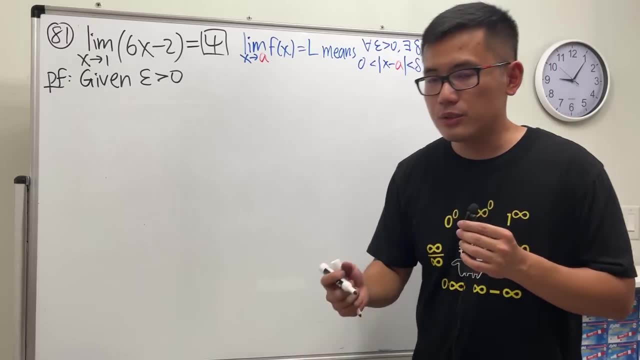 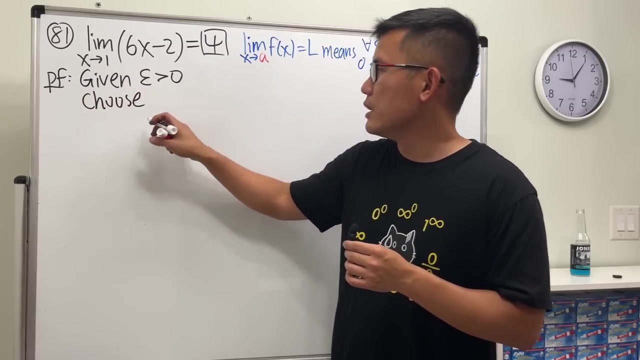 among like 10 points anyway. anyway. next, you see that right here it says there exist. so, to show that there exists, you are going to pick, you are going to select, you are going to choose. uh, i like to use the word choose, so that means you can show that, hey, we do have such a delta. we are going to choose. 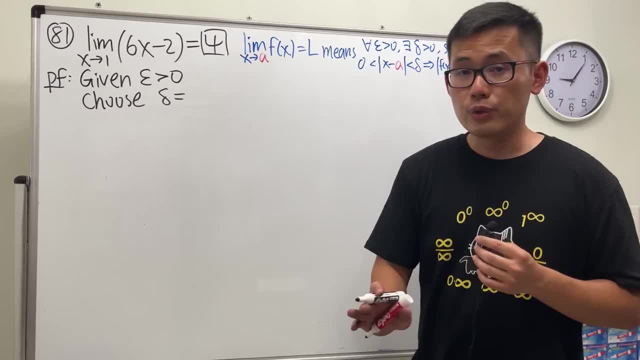 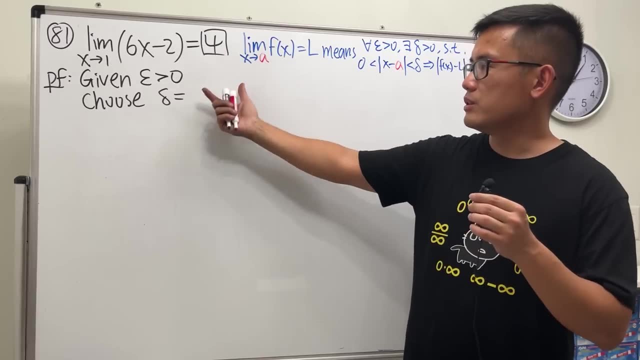 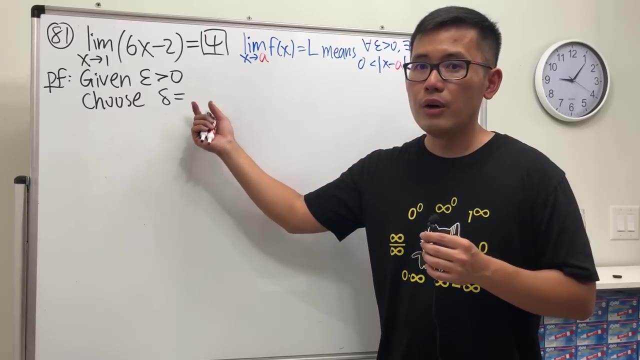 delta. but delta is what we don't know yet. just leave it blank for now. a lot of students get stuck with epsilon delta definitions because they just don't know what delta is, and then they're stuck. i'm telling you, don't worry, just write it down, leave it blank for now and then we'll come. 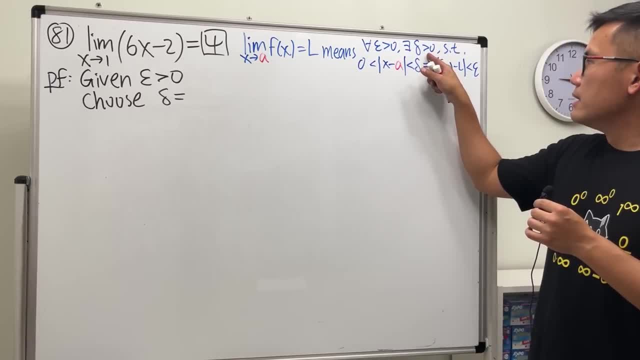 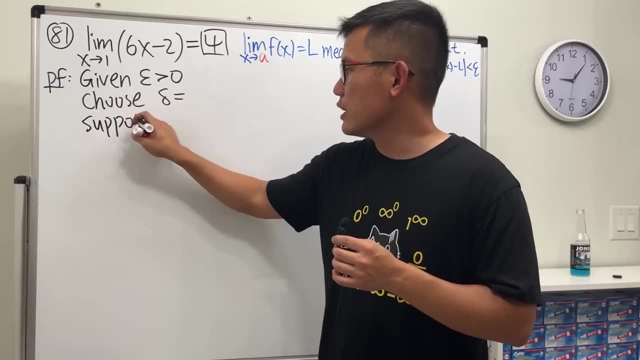 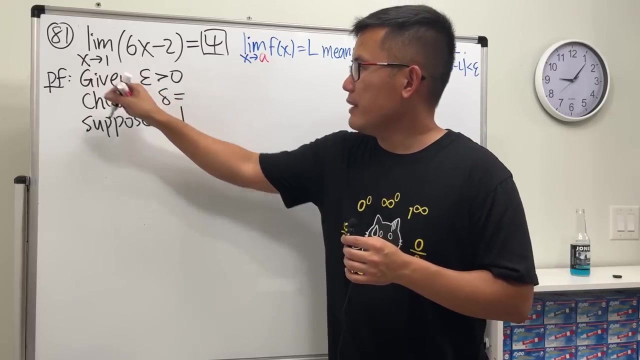 back to you later, okay, okay, such that we are going to assume that we have this. so i'm just going to say, suppose, if you would like, and also say, assume, but suppose, suppose this is true, meaning that the absolute value, and here we have x minus one, right? so we're going to assume that we have x minus one. 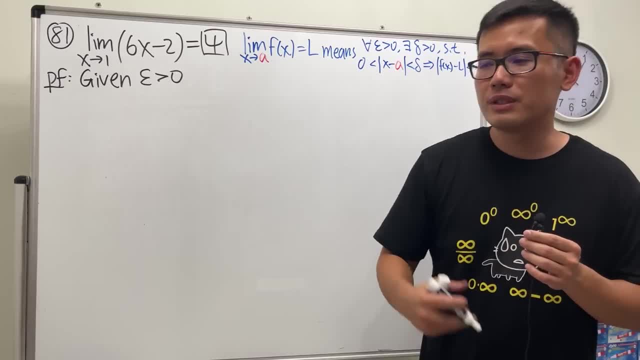 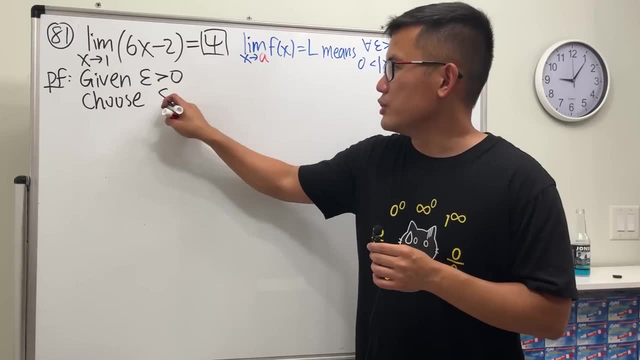 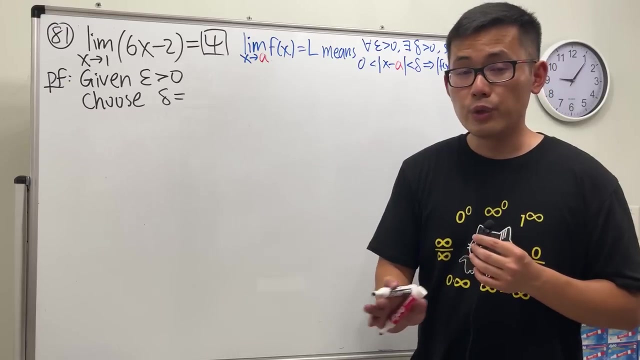 So to show that there exists, you are going to pick, you're going to select, you're going to choose. I Like to use the word choose, So that means you can show the hey, we do have such a Delta, we're gonna choose Delta. but Delta is what we don't know yet. Just leave it blank for now. A lot of students get stuck with Epsilon Delta definitions because 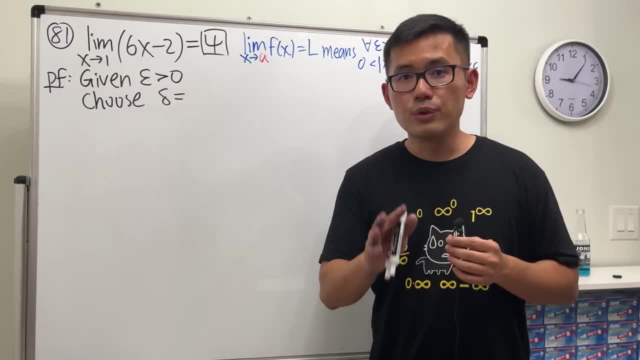 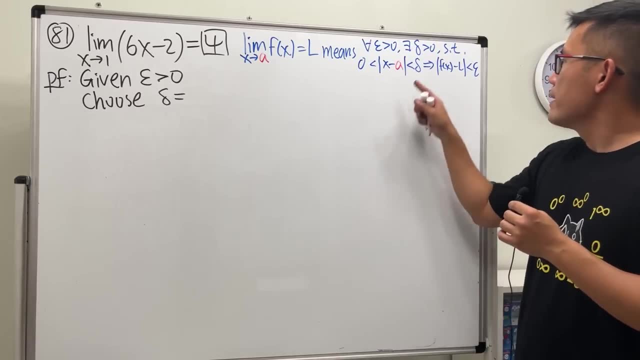 They just don't know what Delta is, and then they're stuck. I'm telling you, don't worry, Just write it down, leave it blank for now, and then we'll come back to you later. Okay, Okay, such that we are going to assume that we have this. 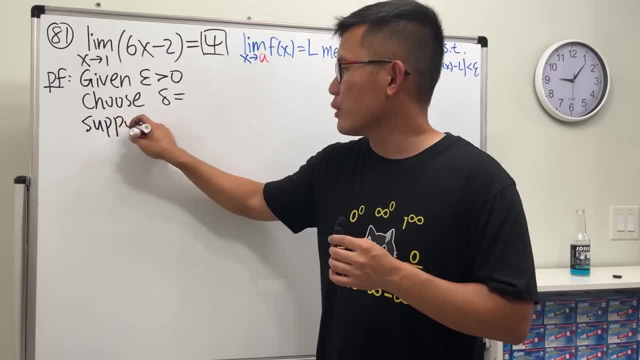 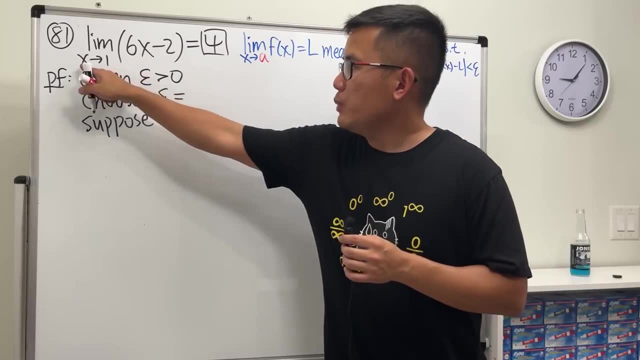 So I'm just gonna say suppose, if you would like, and also say assume. but suppose, Suppose this is true, Meaning that the absolute value, and here we have X minus 1, X minus 1, Because this is x minus a, so it's x minus 1.. 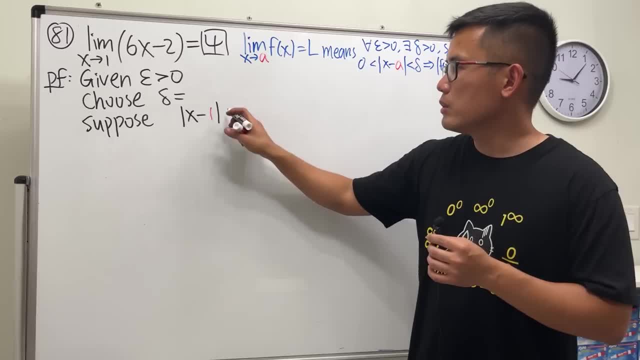 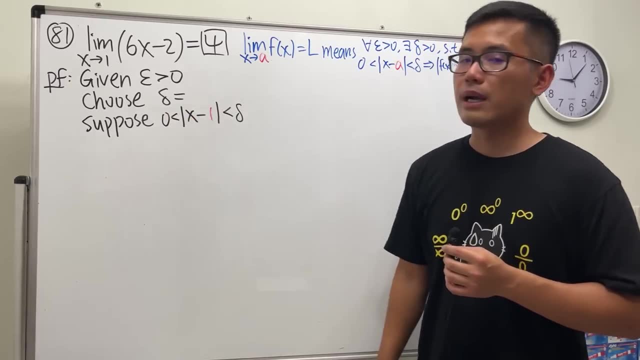 Suppose the distance between x and 1 is small, meaning less than delta, but we don't want x to be 1.. So we put this greater than 0 when you read it backwards Because of this. that's why, 5 hours ago, 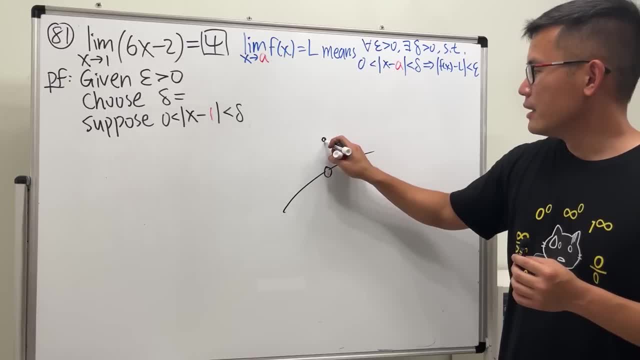 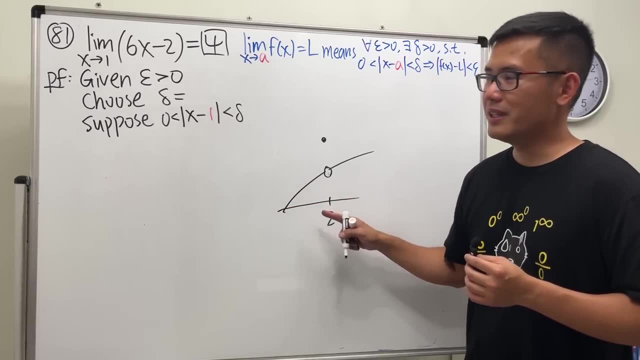 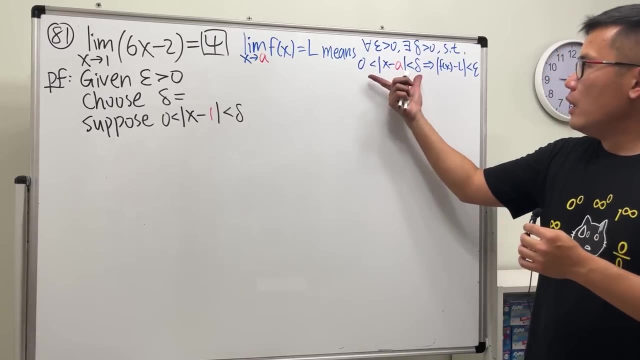 when we saw the graph. you see, we don't care when x is exactly 2 or 3.. We don't care because we have this inequality. Anyway, we assume we suppose we have this condition. With that, we hope to show this is true. 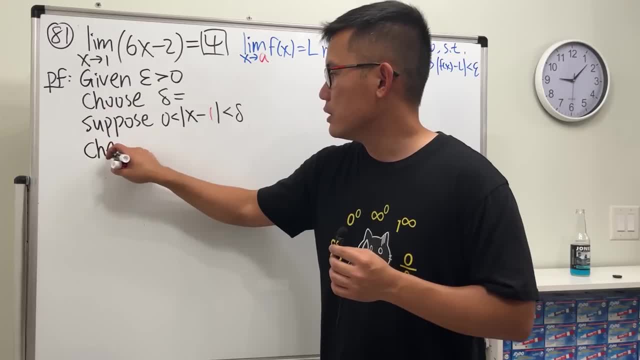 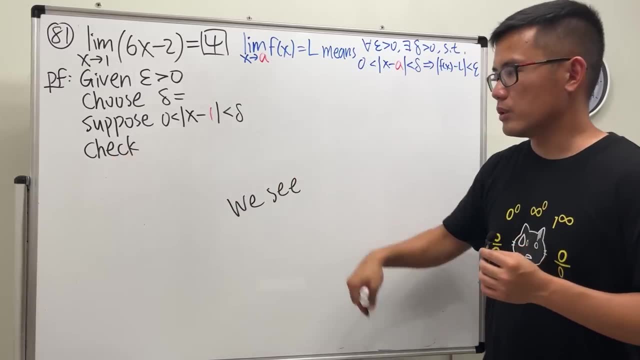 And we hope to show that means we better do the check, So we are going to check. Or you can also say: we see Put, we see here, and then just go ahead and do the computations and all that, But anyway, we check. 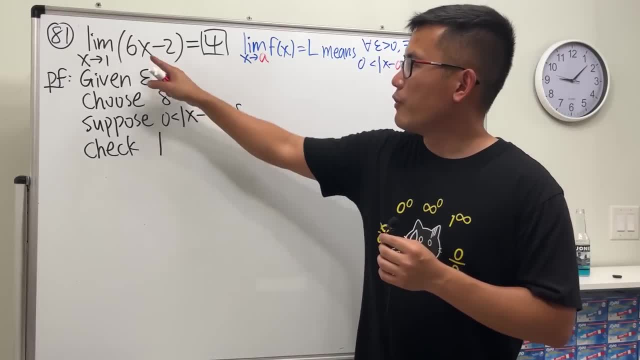 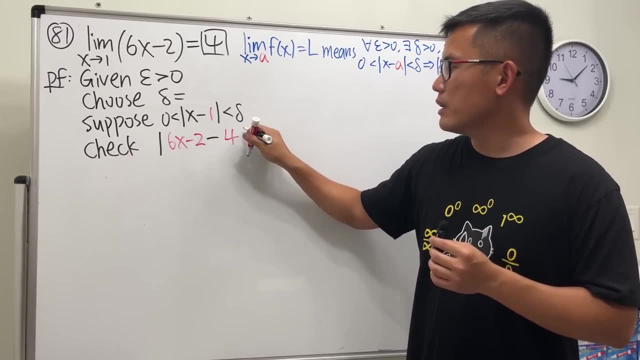 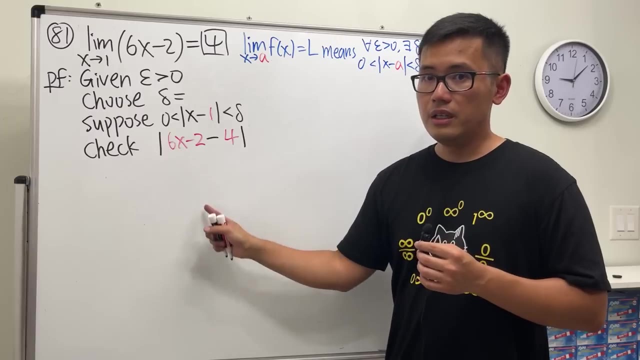 Check what The absolute value, our function is: 6x minus 2.. And then minus the l, which is 4.. Okay, Function minus l. And then we hope to show that this right here is going to be less than epsilon. 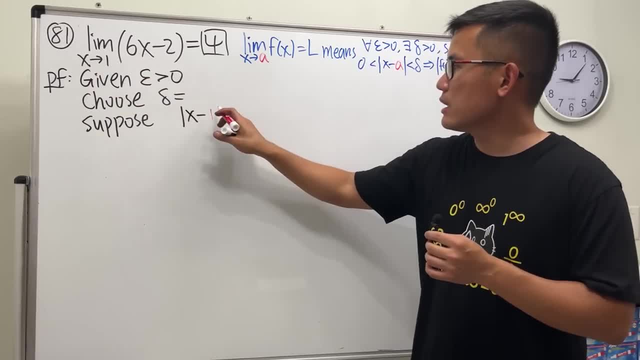 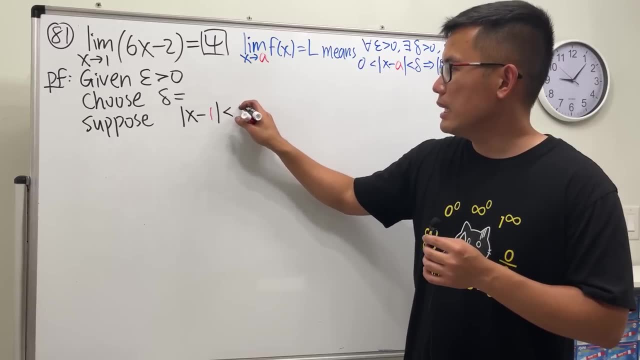 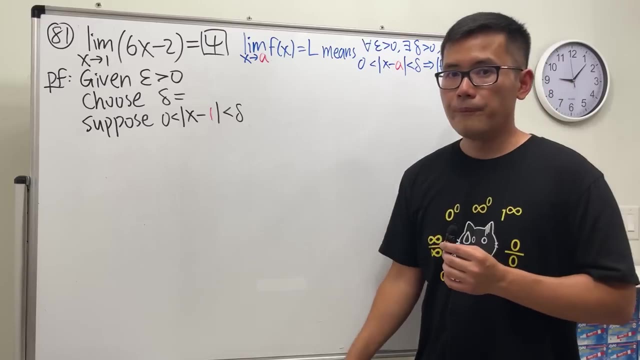 to the x minus one, because this is x minus a, so it's x minus one. suppose the distance between x and one is small, meaning less than delta. but we don't want x to be one. okay, so you put this greater than zero when you read it backwards because of this. that's why, five hours ago, 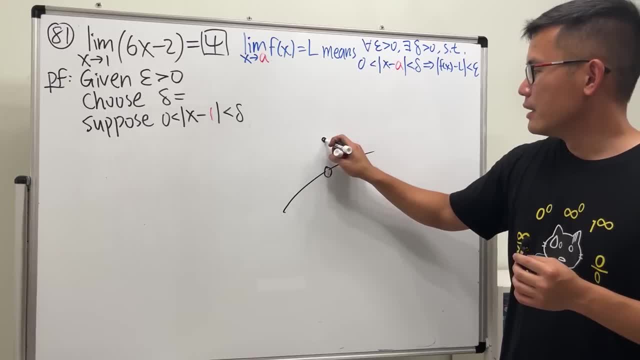 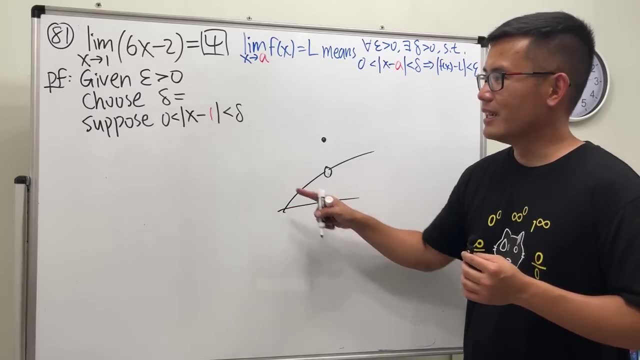 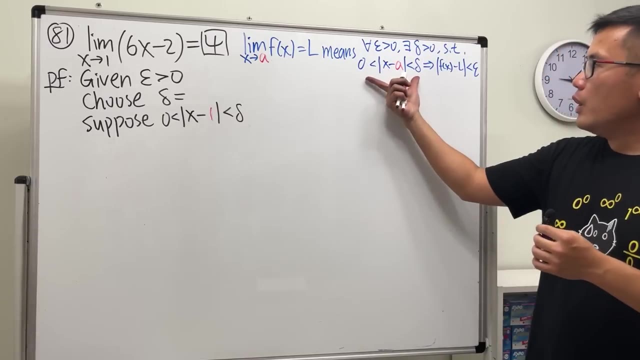 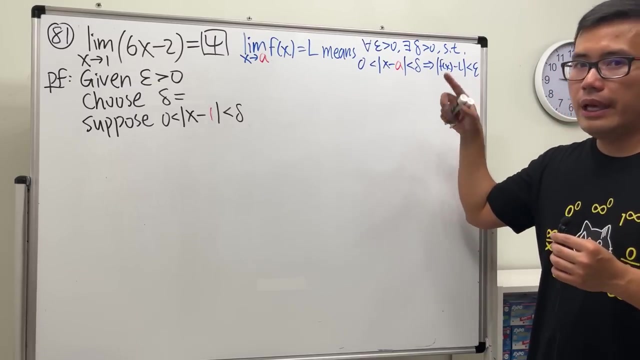 when we saw the graph. you see, we don't care when x is aside two or three, we don't care because we have this inequality. yeah, anyway, we assume we are supposed we have this condition with that. we hope to show this is true, and we hope to show that means we. 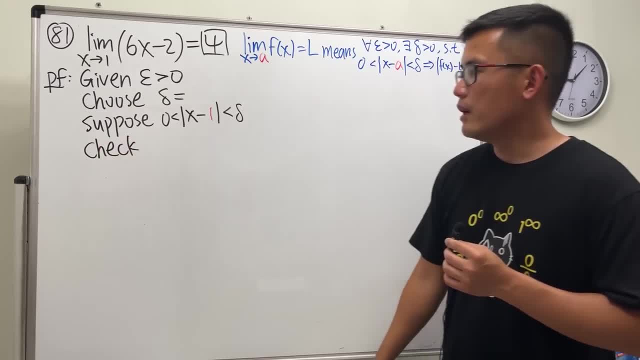 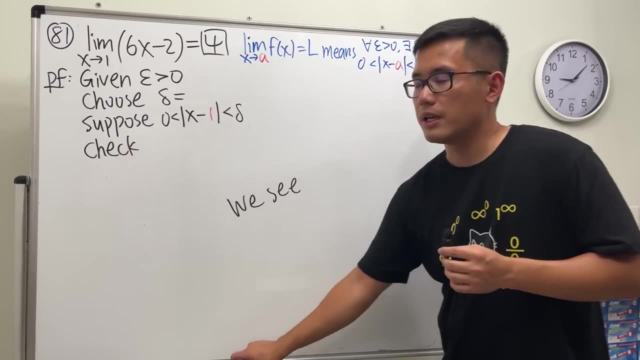 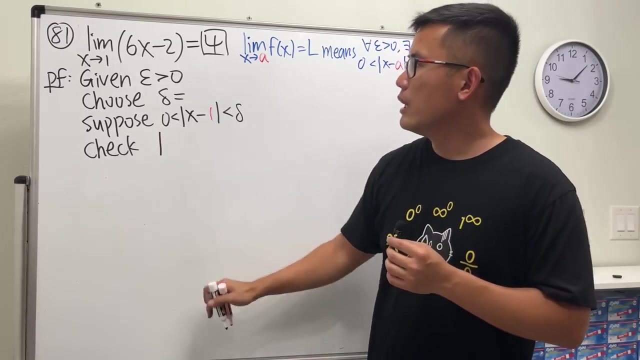 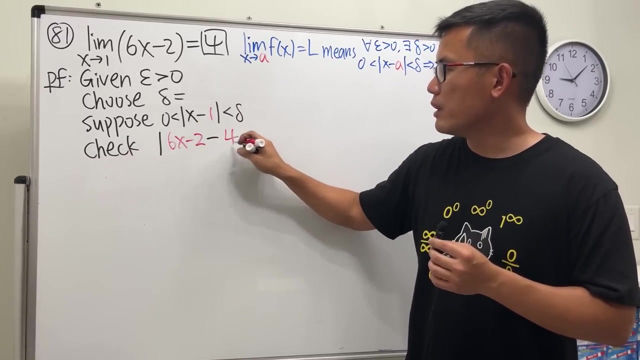 better do the check, so we are going to check. or you can also say: we see who we see here and then just go ahead and do the computations and hold up. by the way, we check. check what the absolute value, our function is: 6x minus 2 and then minus the L, which is 4. okay, function minus L, and then we hope. 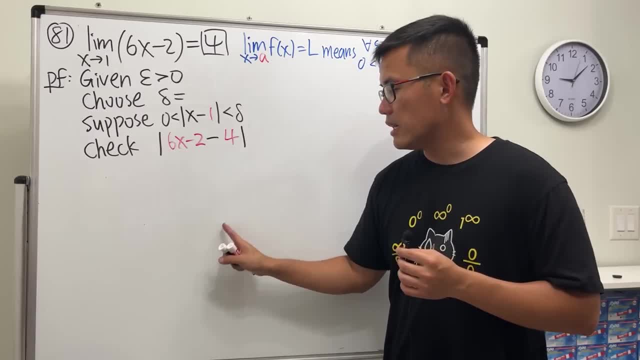 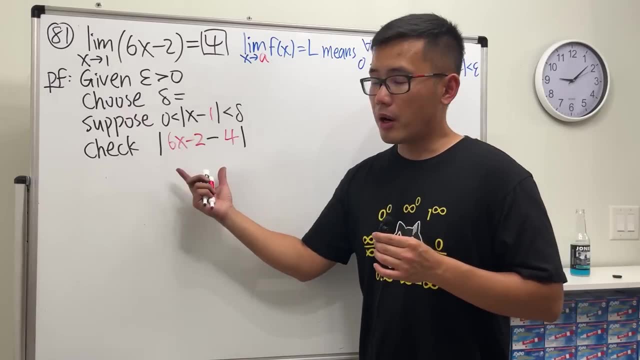 to show that this right here is going to be less than epsilon. okay, so this is the general framework. okay, so this is the general framework. okay, so this is the general framework. now, this is the part that we will have to do. now, this is the part that we will have to do. 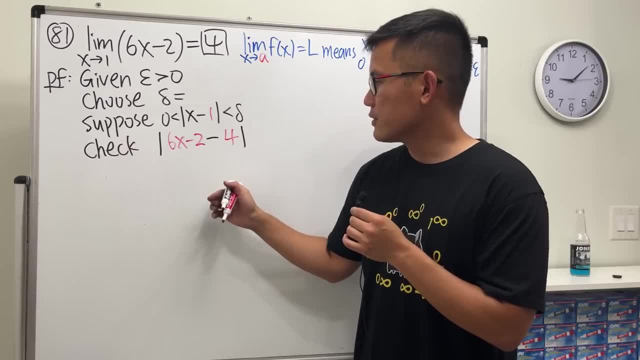 now, this is the part that we will have to do the most amount of work, and then just do some the most amount of work, and then just do some the most amount of work, and then just do some. algebra first minus two minus four is minus six. algebra first minus two minus four is minus six. 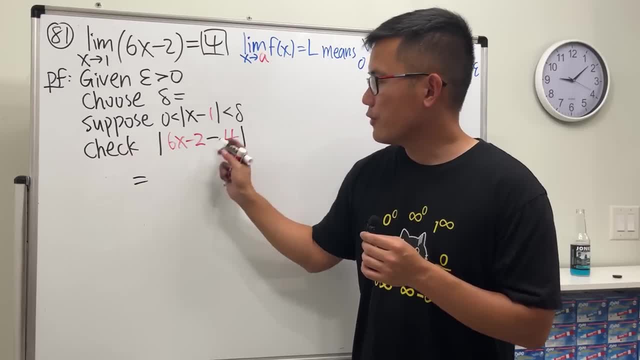 algebra: first minus two minus four is minus six and um we can also factor the six on our side. so and um we can also factor the six on our side. so and um we can also factor the six on our side. so perhaps I'll show you guys, like this six minus. 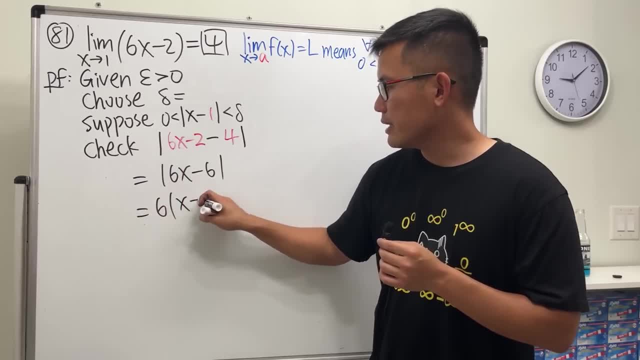 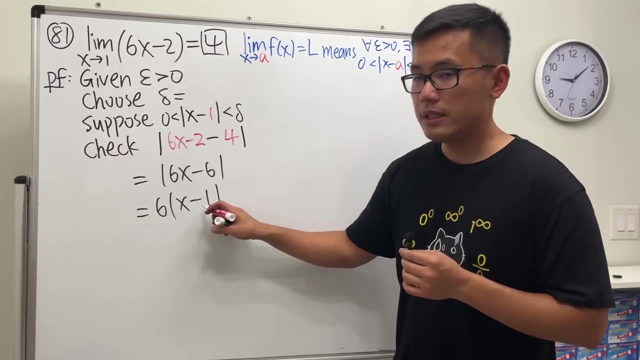 perhaps I'll show you guys like this: six minus. perhaps I'll show you guys like this: six minus six, and then factor all the six and then we get X six. and then factor all the six and then we get X 1. okay, and this is great, because you see how we have the X minus 1 in the absolute. 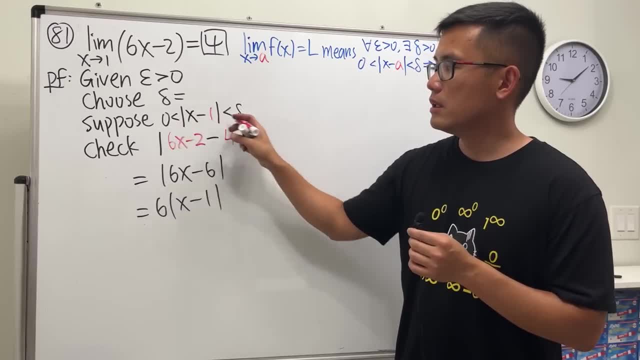 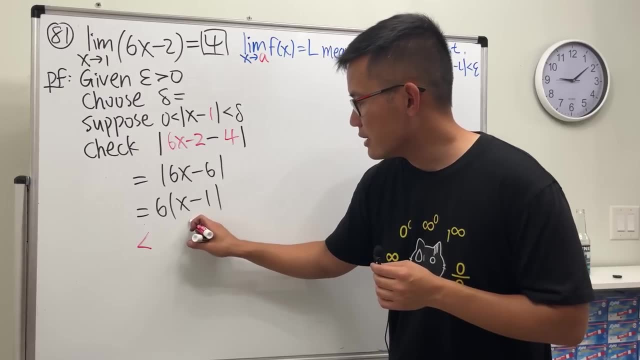 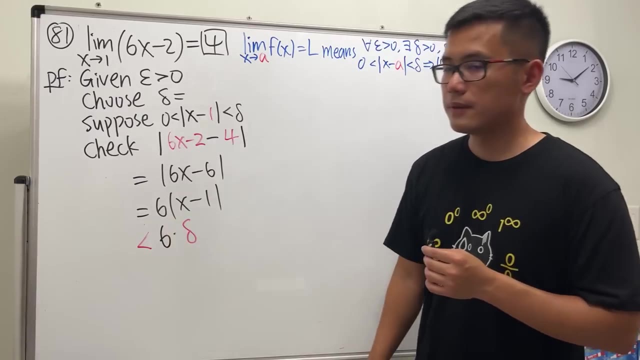 value. we know that right here we have this absolute value of X minus 1 is less than Delta. so we can say that this right here is less than Delta. we replace this absolute value with less than Delta, but we still have the 6 at the front. so you. 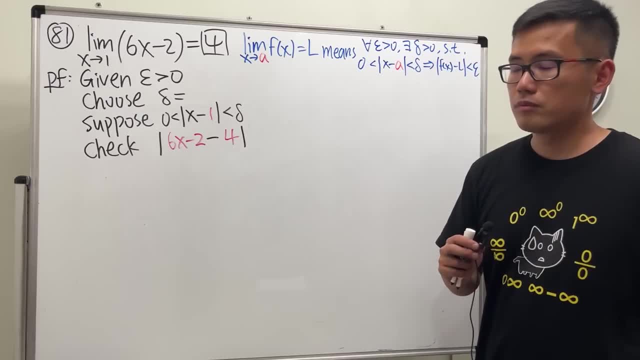 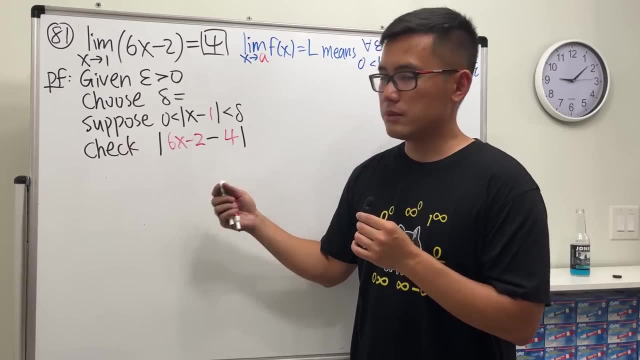 Okay, So this is the general. This is the general rule of frame work. Now, this is the part that we will have to do the most amount of work, And then just do some algebra first. Minus 2 minus 4 is minus 6.. 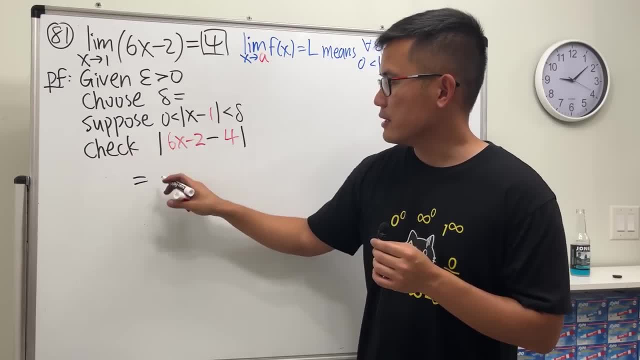 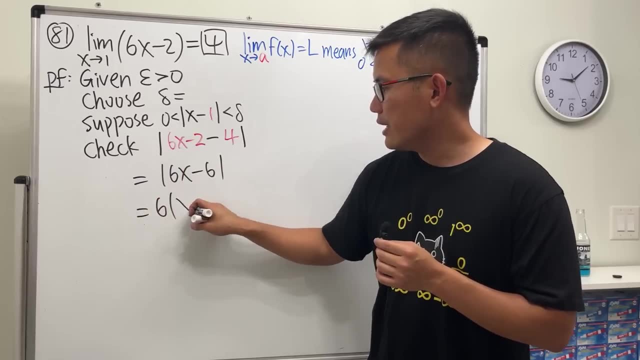 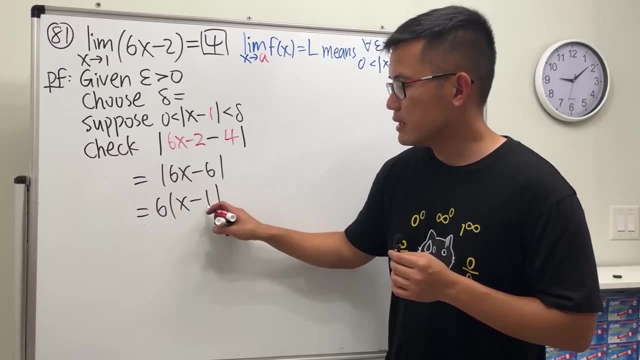 And we can also factor out the 6 on our side. So perhaps I'll show you guys like this: 6x minus 6, and then factor out the 6, and then we get x minus 1.. Okay, And this is great, because you see how we have the x minus 1 in the absolute value. 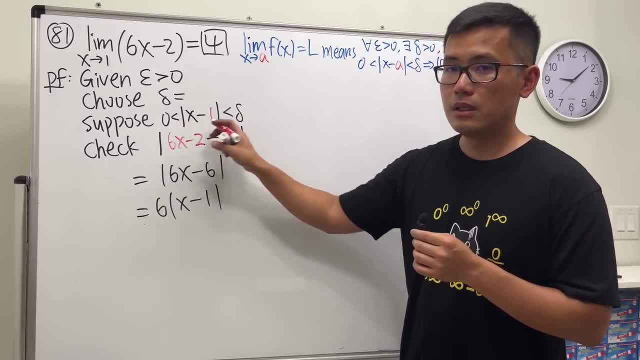 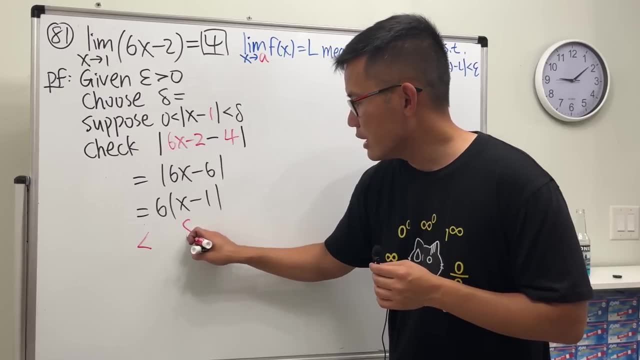 We know that right here we have this: Absolute value of x minus 1 is less than delta. So we can say that this right here is less than delta. We replace this absolute value with less than delta, But we still have the 6 at the front. 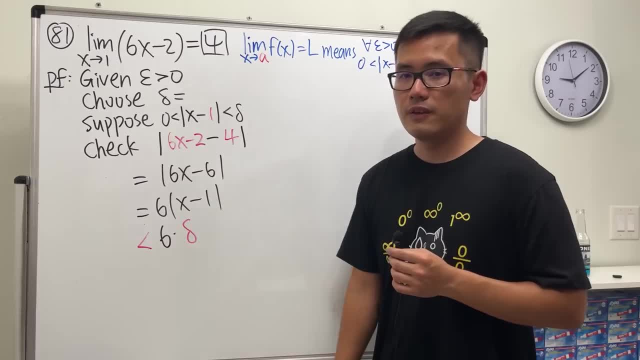 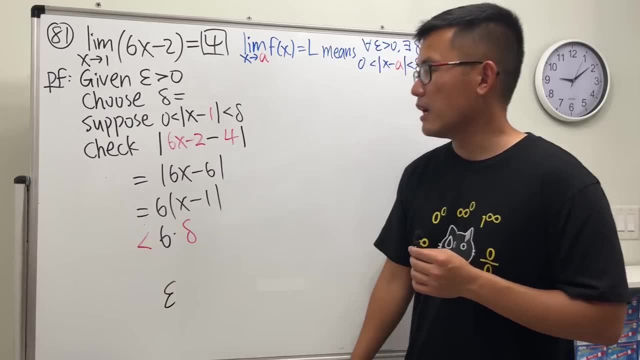 So, you see, we create this inequality. the less than that we want, Very nice. But keep in mind though, at the end we want to end up with what We want, to end up with just epsilon. We just want to end up with epsilon. 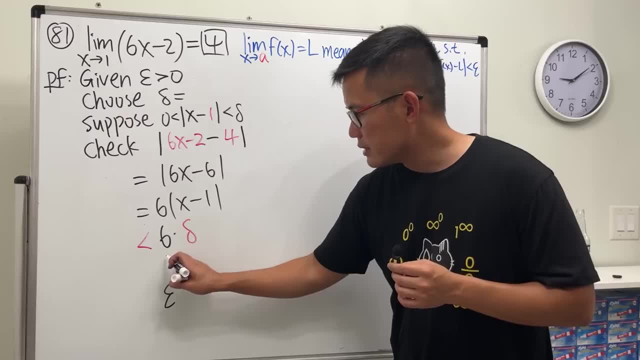 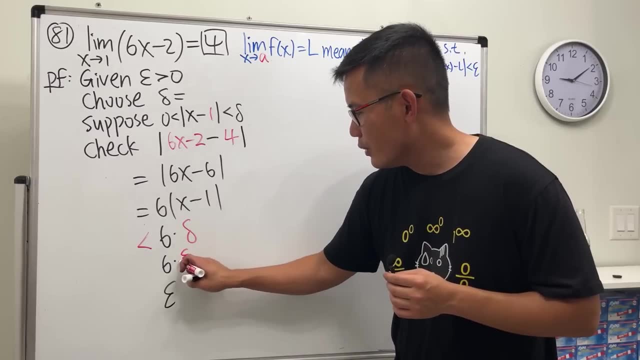 So what do we need? Well, check this out. This right here is 6.. 6 times what will give us epsilon? Well, it's just epsilon over 6, isn't it? Because when we have that, check this out, 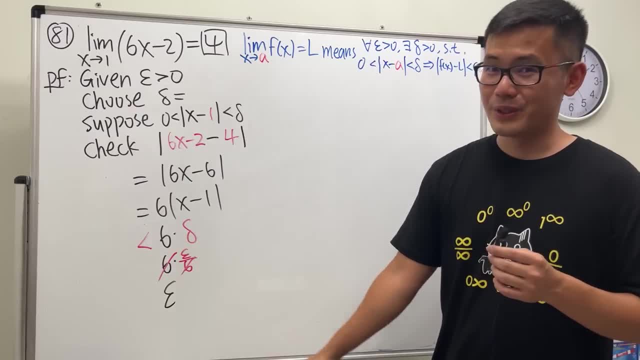 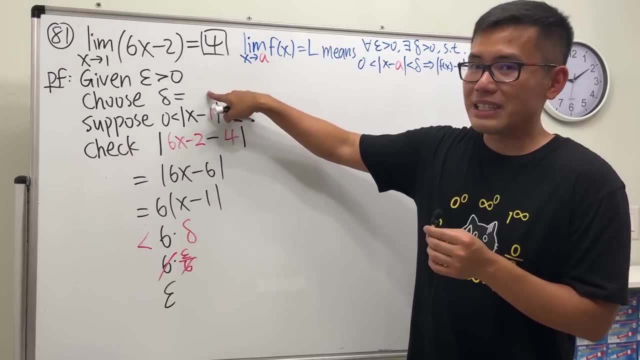 6 and 6 cancel, and then we get the epsilon. Cool huh. So once we figure this out, you see, delta is just epsilon over 6.. We rush back to here and then let's write it down. Let's write down: epsilon over 6.. 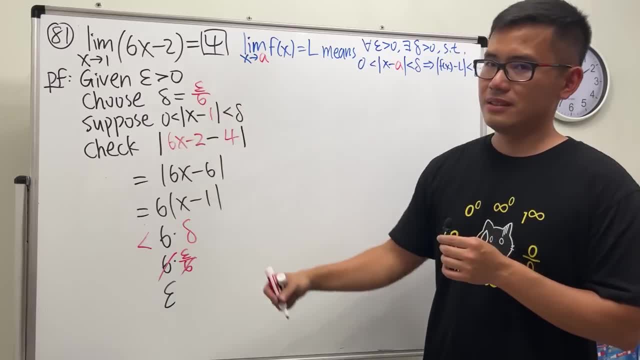 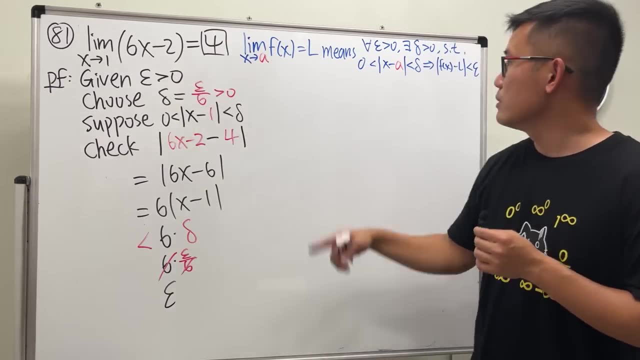 And you see, because epsilon is greater than 0, and over 6 is still greater than 0, so if you would like, you can indicate that, But nobody really does that. We just want to say delta is greater than 0.. 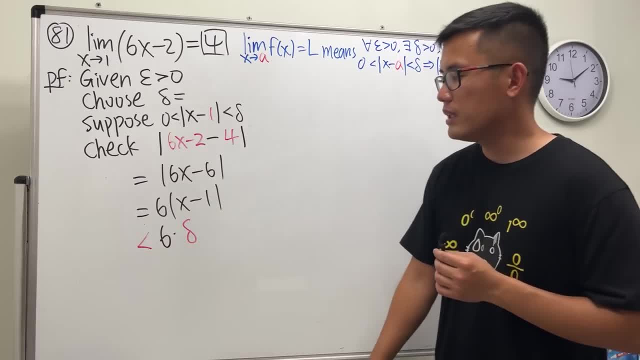 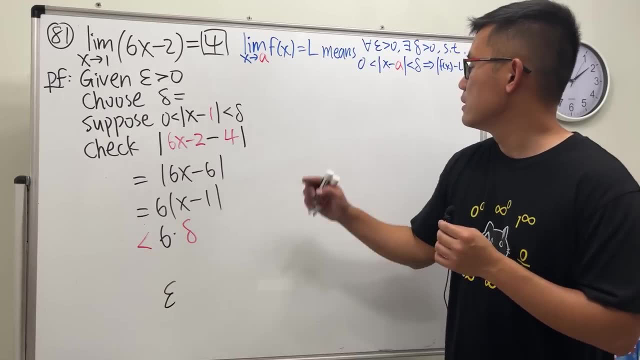 see, we create this inequality. the less than that we want, very nice. but keep in mind though, at the end we want to end up with what we want, to end up with just epsilon. we just want to end up with epsilon. so what do we need? well, check. 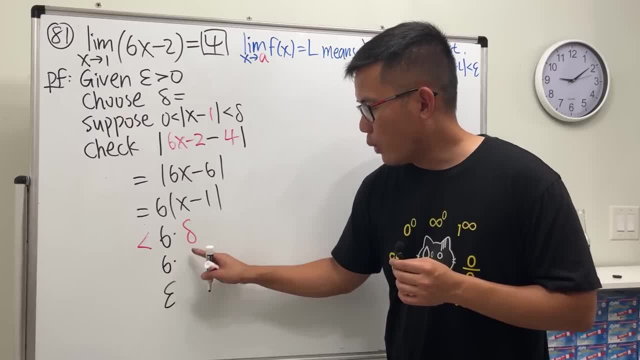 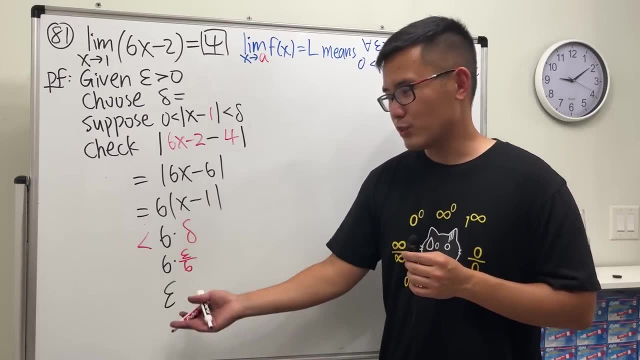 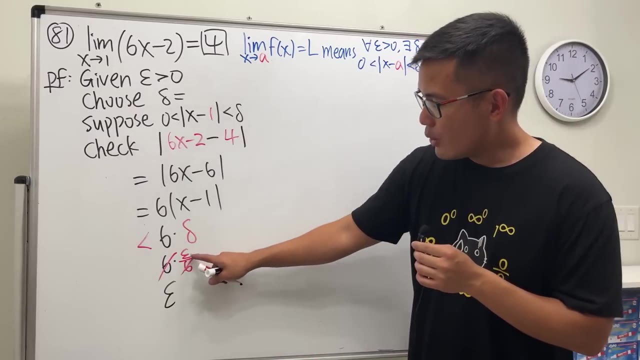 this out. this right here is 6, 6 times what will give us epsilon. well, it's just epsilon over 6, isn't it? because when we have that, check this out, 6 and 6 cancel, and then we get the epsilon, cool huh. so once we figure this out, you see, Delta is just epsilon over 6. we. 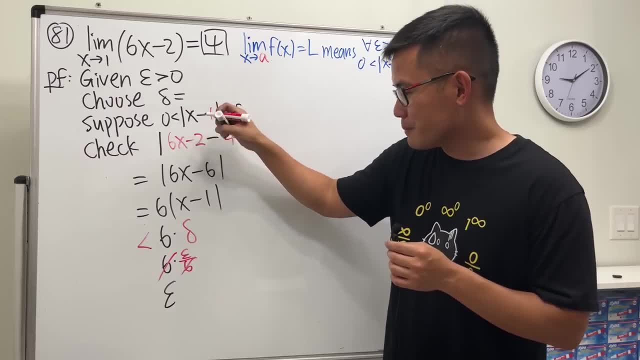 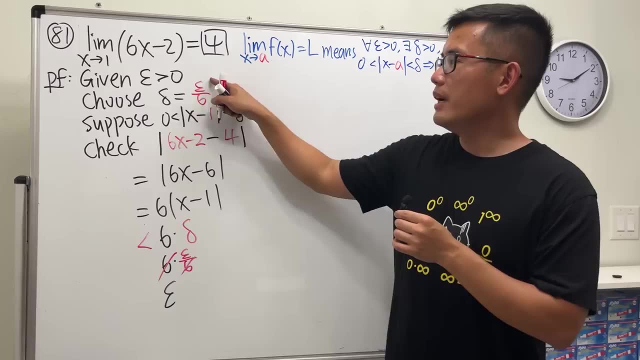 rush back to here and then let's write down. let's write down epsilon over 6, and you see, because epsilon is greater than 0 and over 6 is still greater than 0. so if you would like an indicator, but nobody really does that, yeah, I just want. 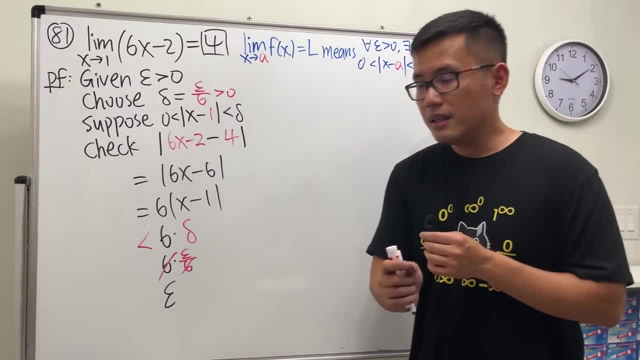 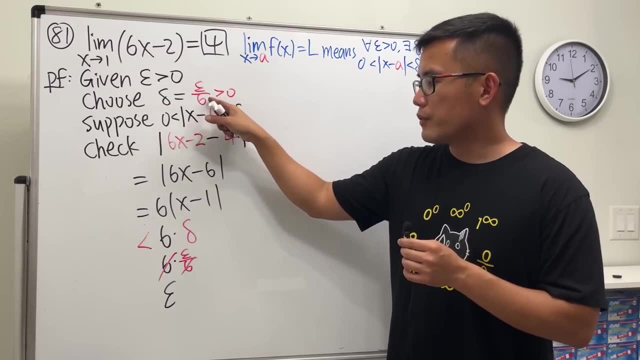 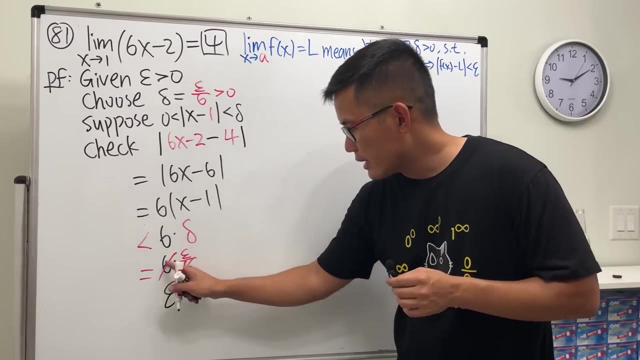 to say Delta is greater than 0. okay, and a few things, though. you see how we pick Delta to be exactly. we pick Delta to be equal to epsilon over 6. so right here I'm going to put on equal sign: Delta is equal to epsilon over 6, and I cancel. 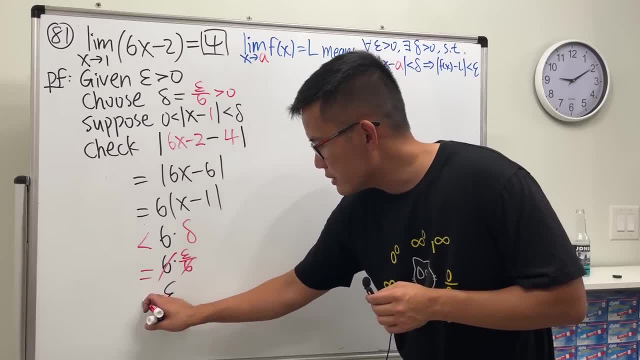 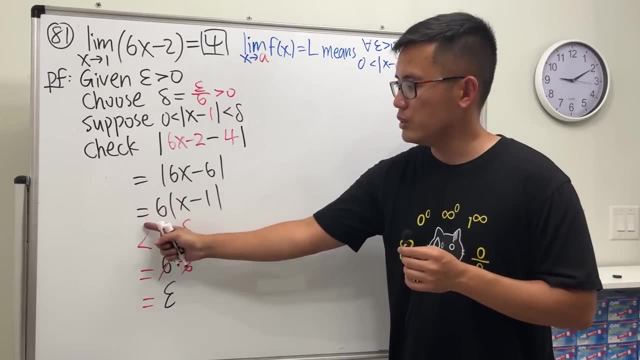 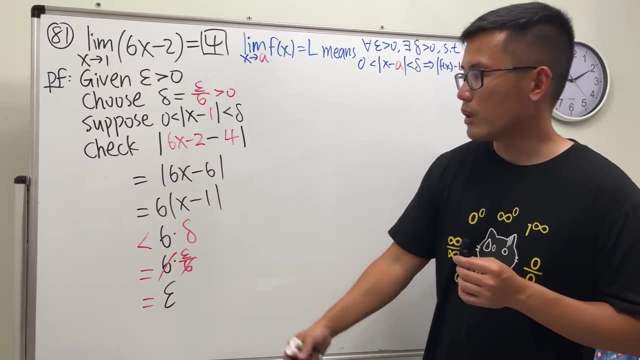 cancel. so, after the simplification, this right here is still equal. but the way that you read this is that we have this inequality, which is equal to this, which is equal to that, and then this is less than this and this is equal to that, is equal to that, in another word. 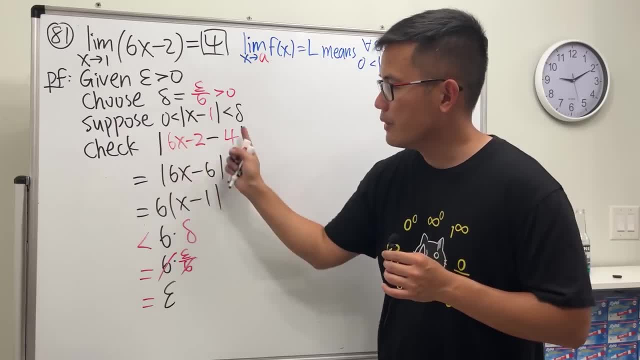 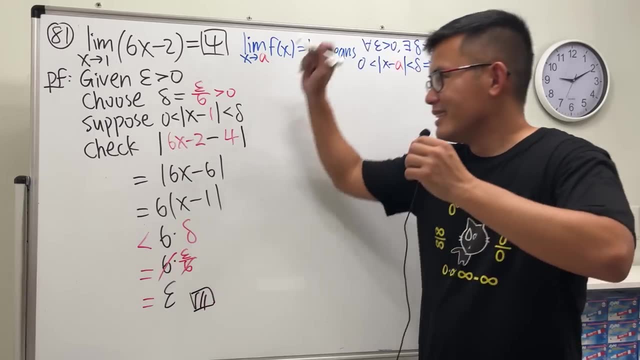 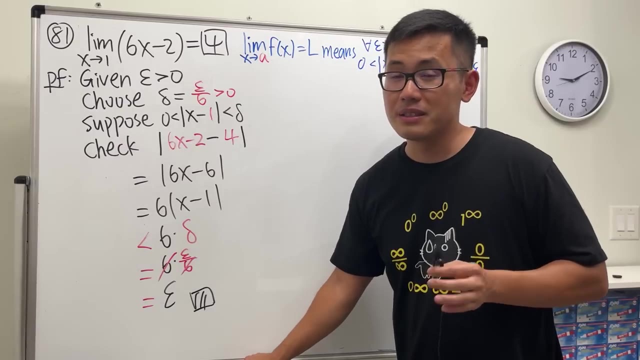 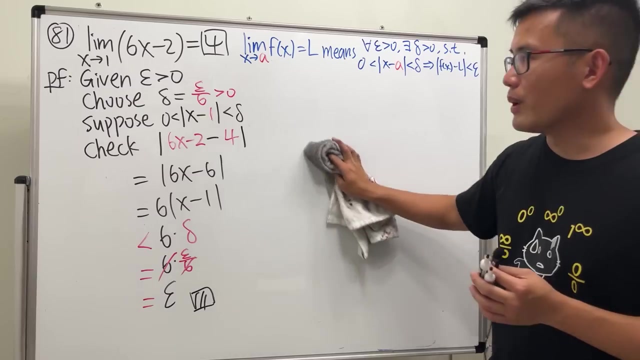 this inequality. sorry, this absolute value is less than epsilon, so we are done. put box: yay, 20 more questions. it might be confusing the first few times that we're doing it. that's what we're doing 10 times okay, so let's try another one. I'm going to erase everything, not that. all right, okay, let's. 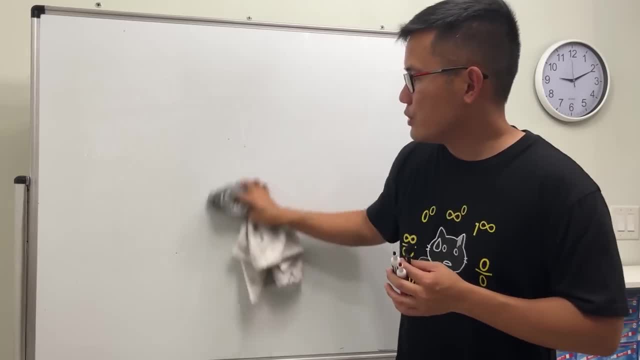 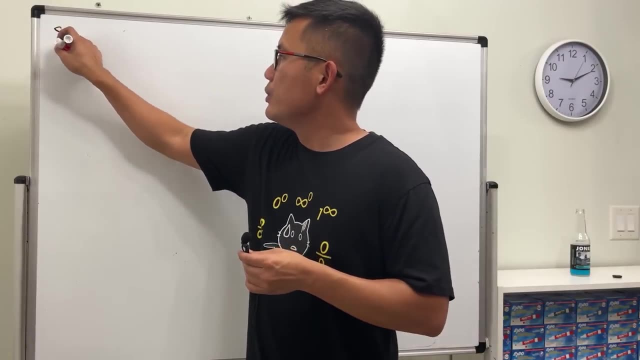 Let's erase this as well- Why I want to show you guys- The more you write it down, the better that we remember it. Okay, let's try another one, Number 82.. Here we have the limit, And then we have x approaching negative 2.. 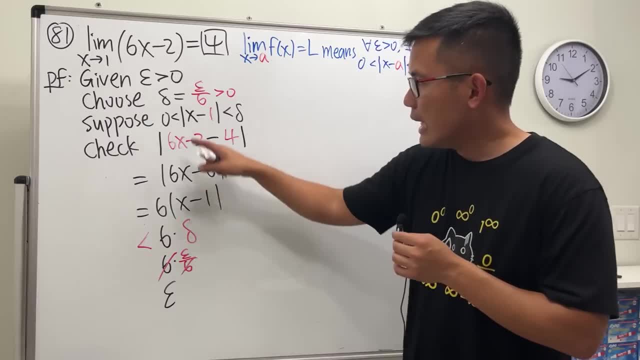 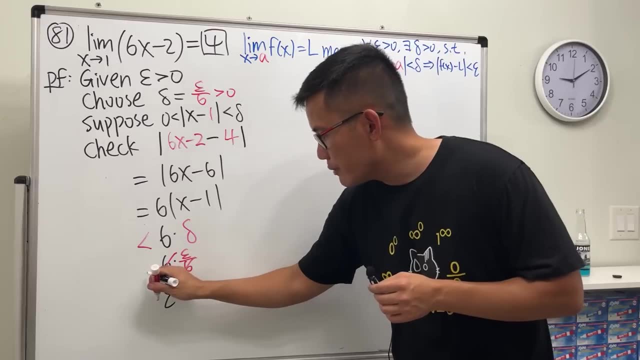 Okay, And a few things, though. You see how we pick delta. to be exactly, We pick delta to be equal to epsilon over 6.. So right here I'm going to put an equal sign: Delta is equal to epsilon over 6.. 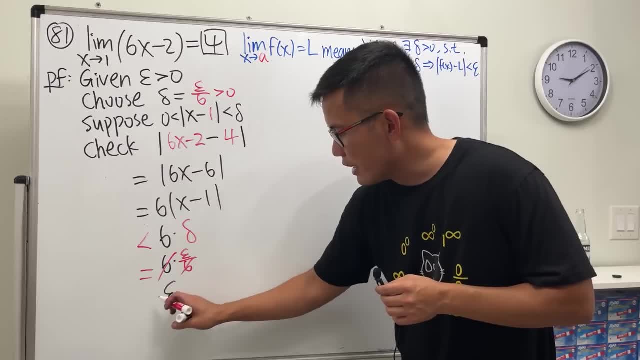 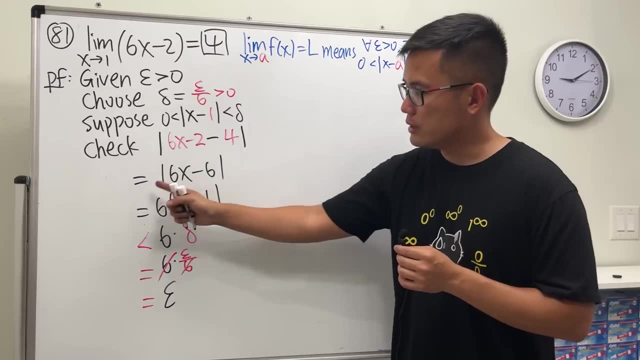 And I cancel, cancel. So, after the simplification, this right here is still equal. But the way that you read this is that we have this inequality, which is equal to this, which is equal to that, and then this is less than this. 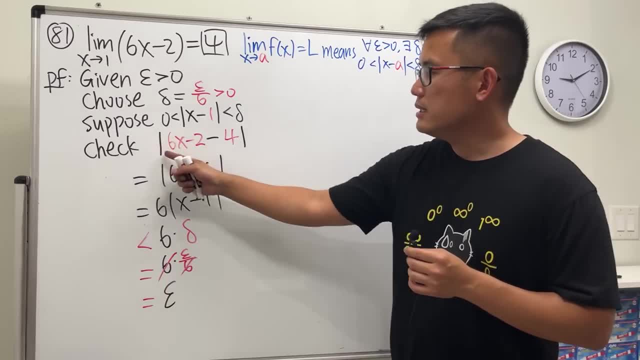 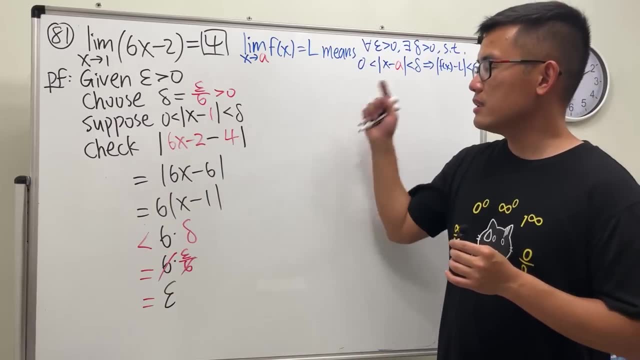 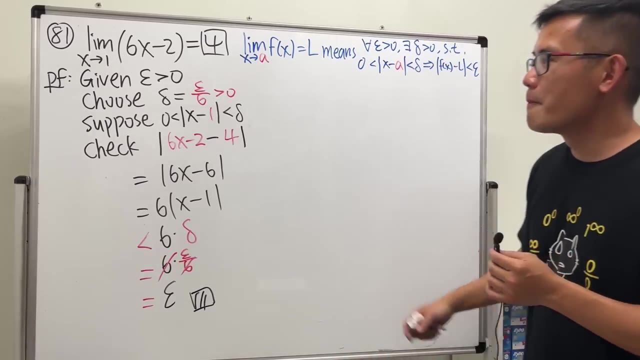 And this is equal to that. it's equal to that In another word, this inequality. Sorry, this absolute value is less than epsilon, So we have that. Put a box. Yay, 20 more questions. It might be confusing the first few times that we're doing it. 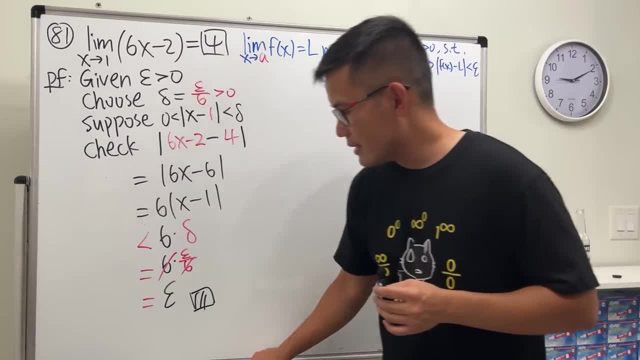 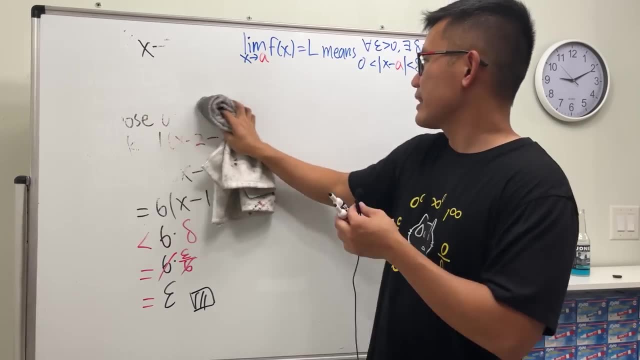 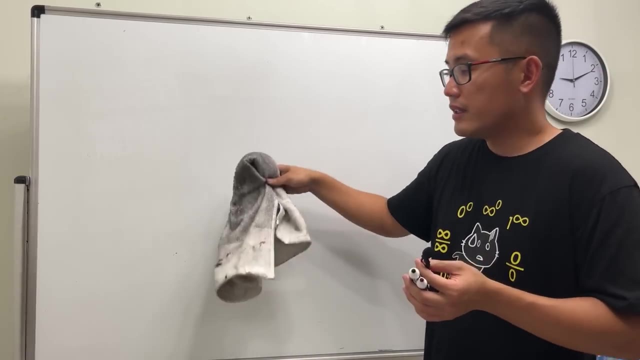 That's why we're doing it 10 times, Okay, So let's try another one. I'm going to erase everything, Not that, Okay, let's erase this as well- Why I want to show you guys- The more you write it down, the better that we remember it. 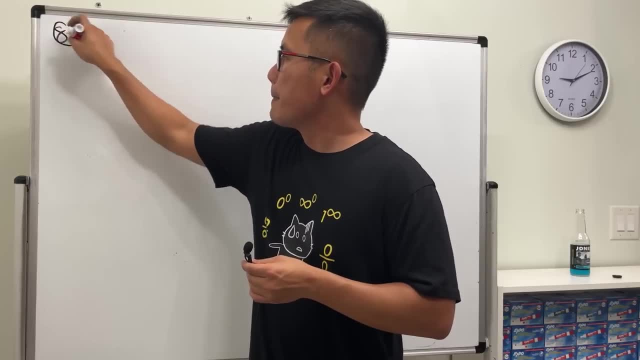 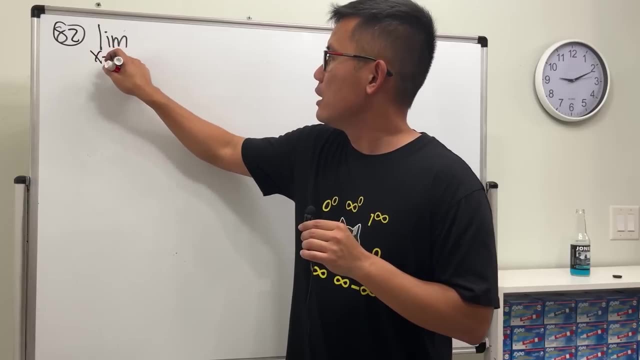 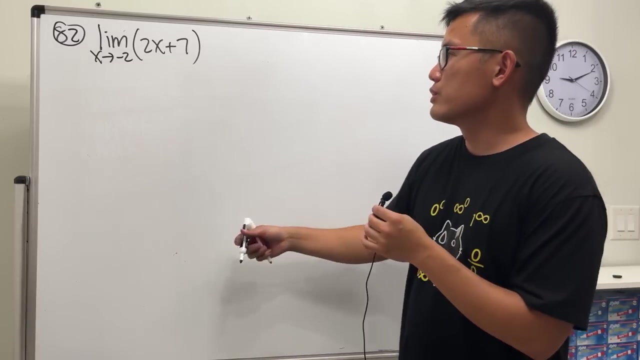 Okay, let's try another one, Number 82. Here we have the limit, and then we have x approaching negative 2, and then 2x plus 7.. Okay, and then to do this? you can just do this in your head. 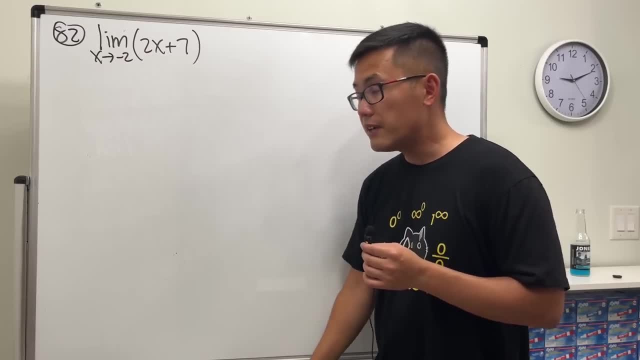 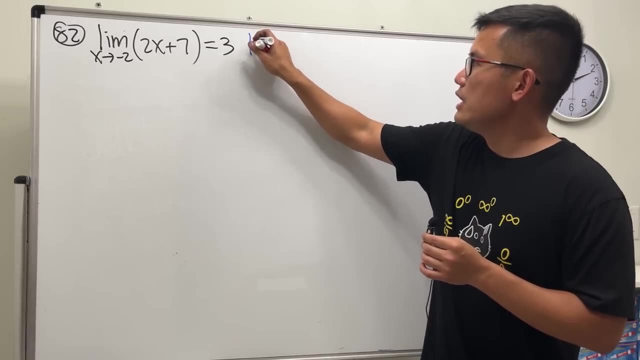 Negative 2 here 2 times negative 2 is negative 4, plus 7 is 3.. So this right here is equal to 3.. Done Now. epsilon delta definition means if we have the limit and if x is. 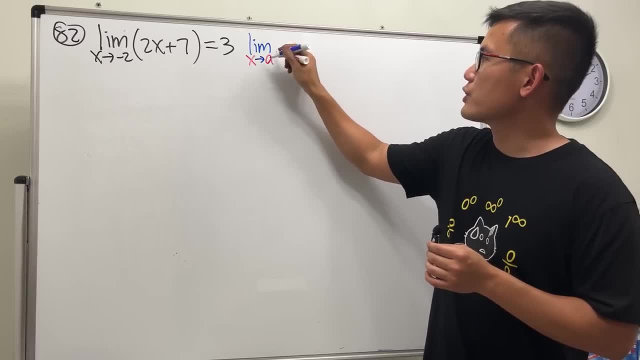 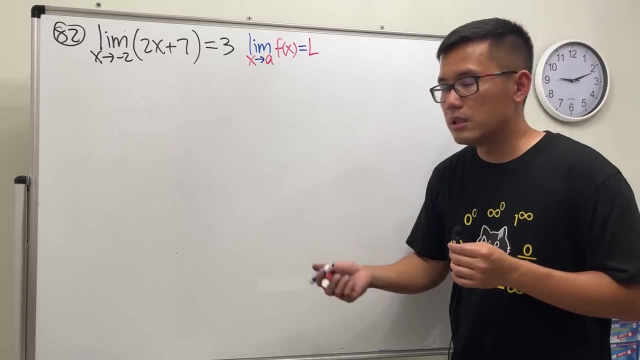 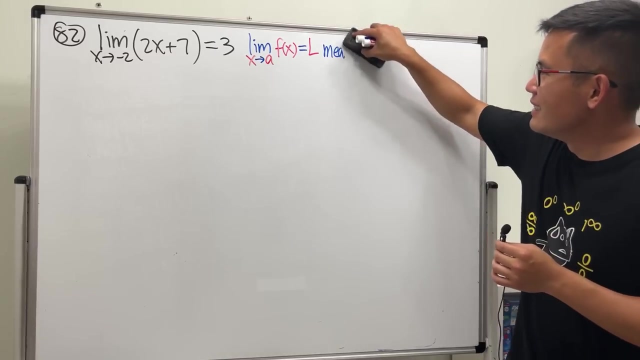 Approaching a. If we have a function f of x, If this right here give us a limit, let's call it L. This right here means No, not Where's the N? huh. This right here means Here we go. 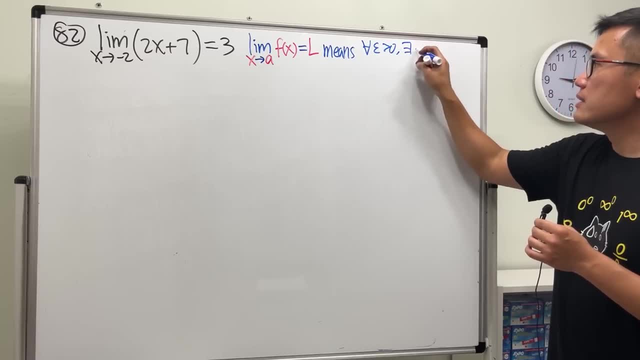 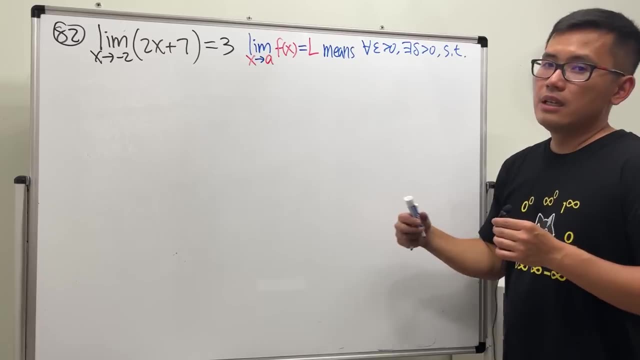 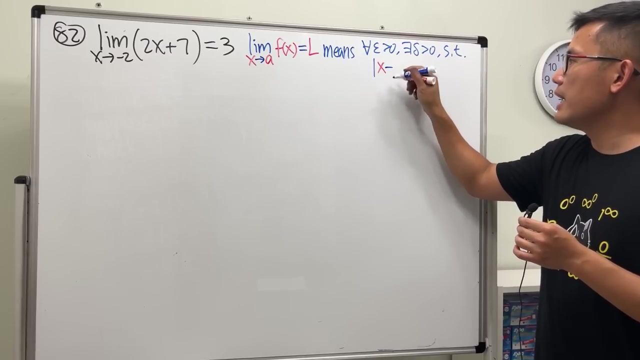 For all epsilon greater than 0, there exists a delta greater than 0,, such that If the distance between x and a is less than delta but bigger than 0, so we write it as absolute value of x minus a is less than delta. 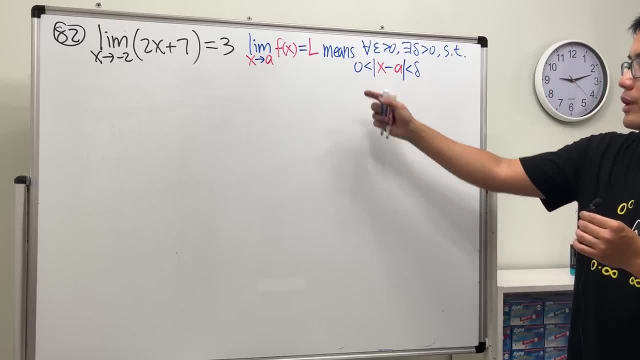 but we don't want x to be a, so we put greater than 0. This right here, implies that's the symbol for. implies implies that the distance between f of x and L is less than epsilon. So we write f of x. 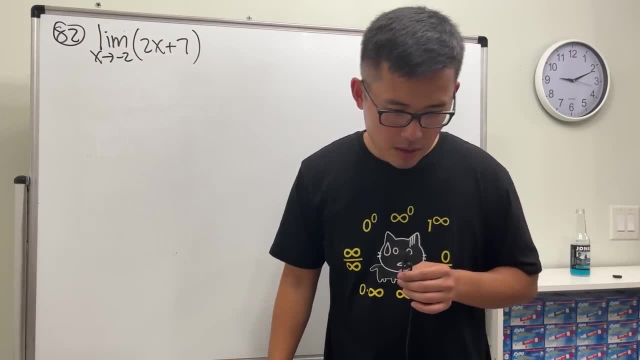 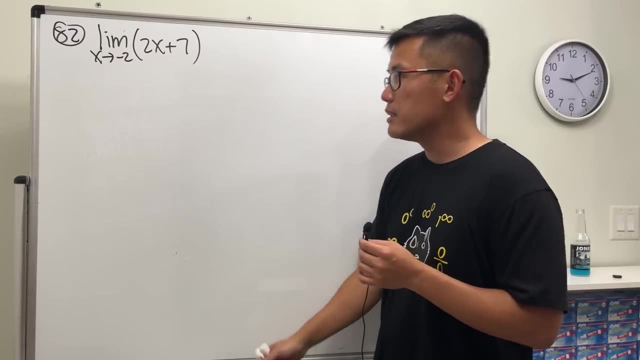 And then 2x plus 7.. Okay, and then to do this, you can just do this in your head: Negative 2 here, 2 times negative, 2 is negative 4, plus 7 is 3.. So this right here is equal to 3.. 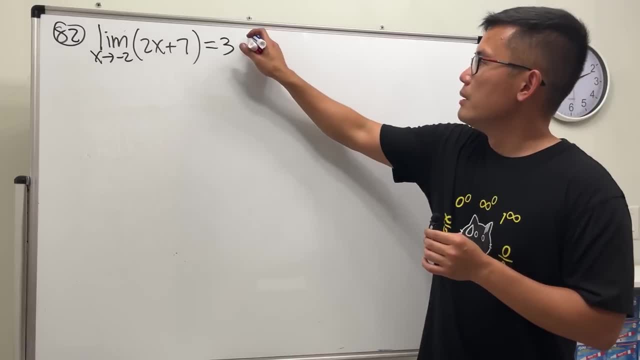 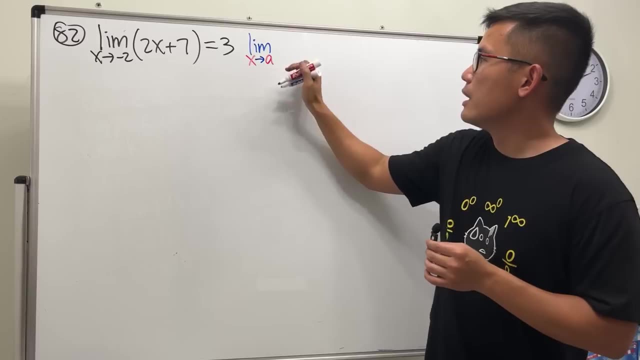 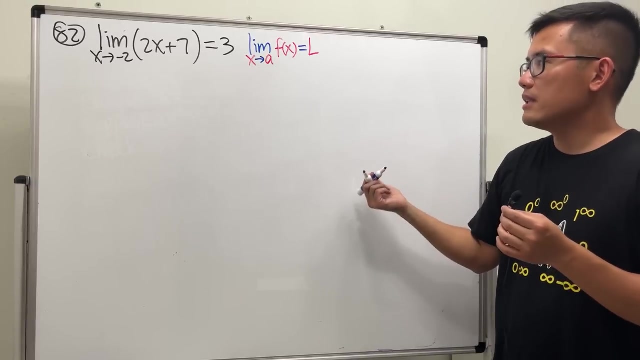 Done Now. epsilon delta definition means: if we have the limit and if x is approaching a, if we have a function f of x, if this right here gives us a limit, let's call it L. this right here means no, no. 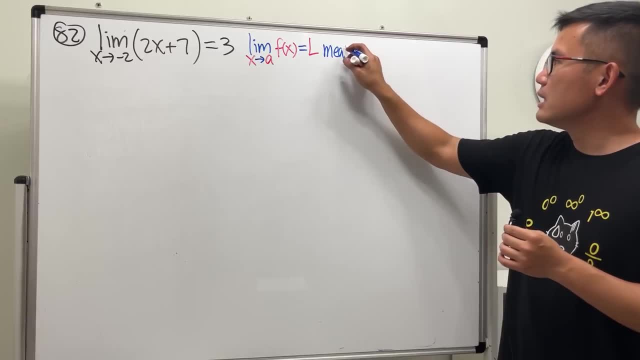 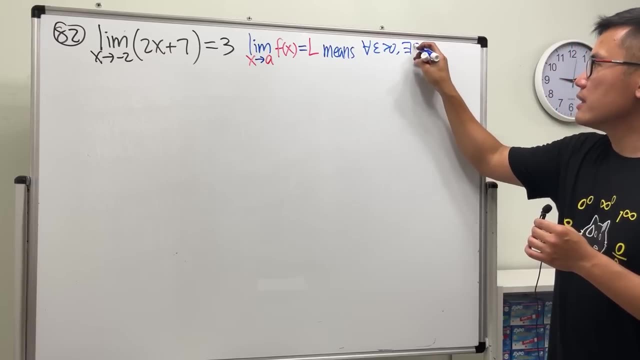 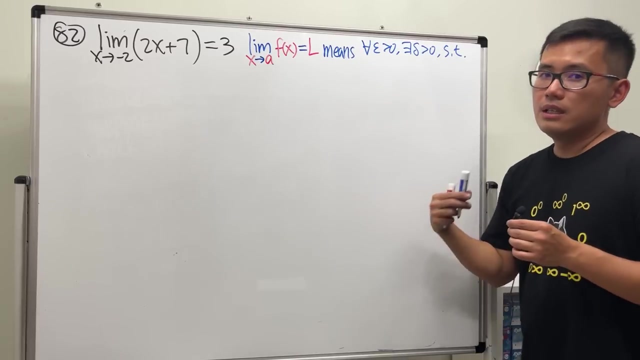 where's the n? huh? This right here means here we go For all epsilon greater than 0, there exists a delta greater than 0,, such that if the distance between x and a is less than delta but bigger than 0,. 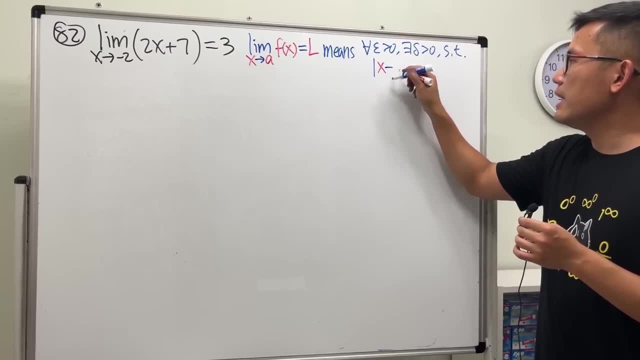 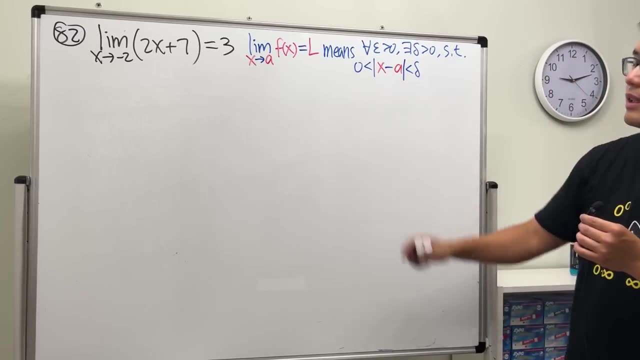 so we write it as absolute value of x minus a is less than delta. but we don't want x2, so we put greater than 0. This right here, implies that's the symbol for. implies implies that the distance between f of x and L is less than epsilon. 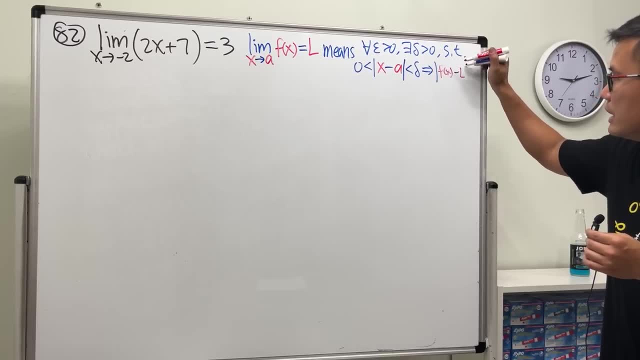 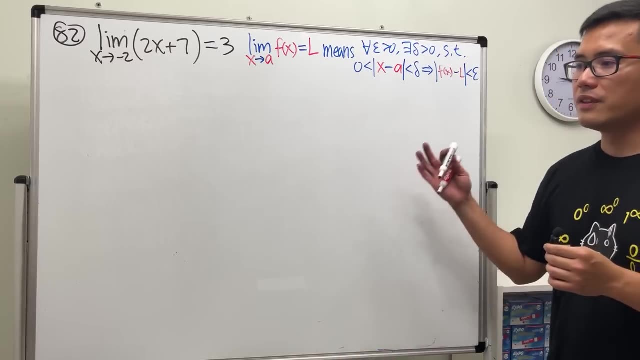 So we write: f of x minus L is less than epsilon. So just go ahead and write down a few more times and then watch the video where I showed you guys an actual example with picture, with number, and then you will see that. 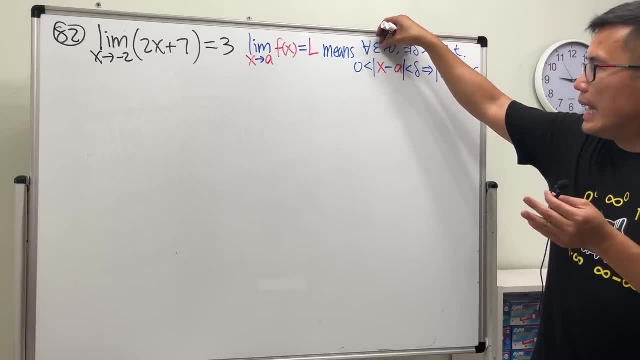 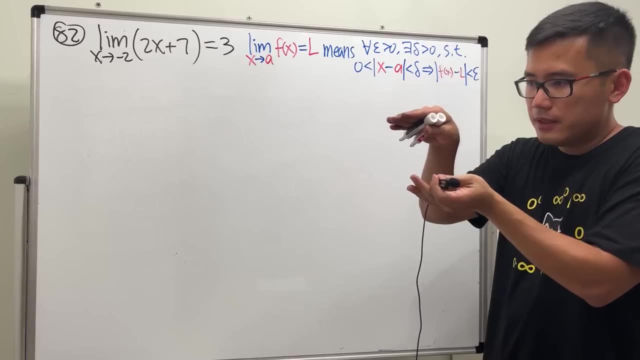 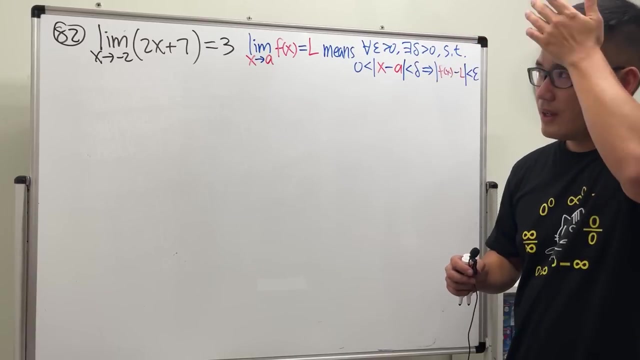 It's like the epsilon stands for error. that's why it's E epsilon. It's kind of like it's squeeze, the, just like kind of make the function as close to the limit as possible, that kind of thing. All right, so now here we go. 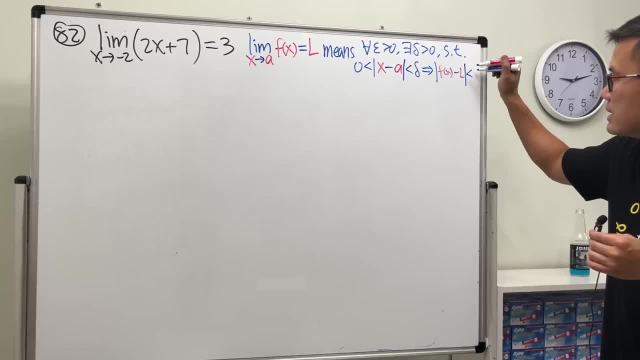 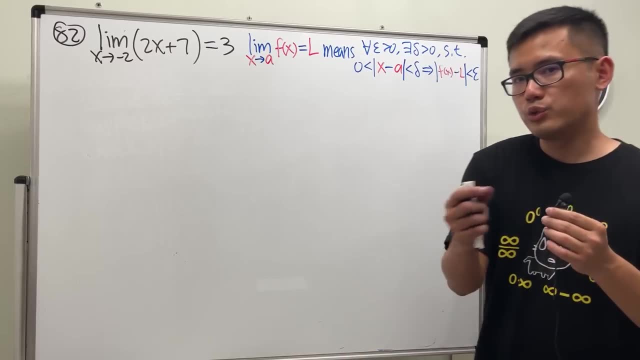 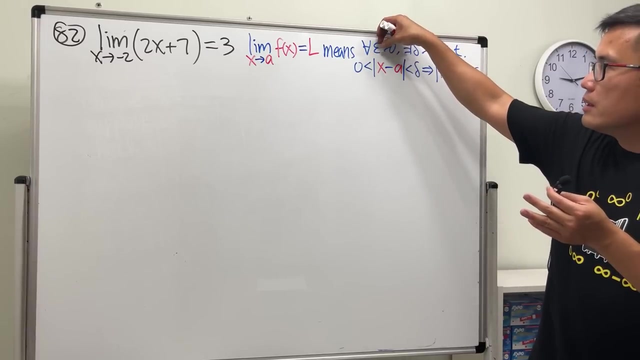 minus L is less than epsilon. So just go ahead and write down a few more times and then watch the video where I showed you guys an actual example with picture, with number, and then you will see that it's like the epsilon stands for error. 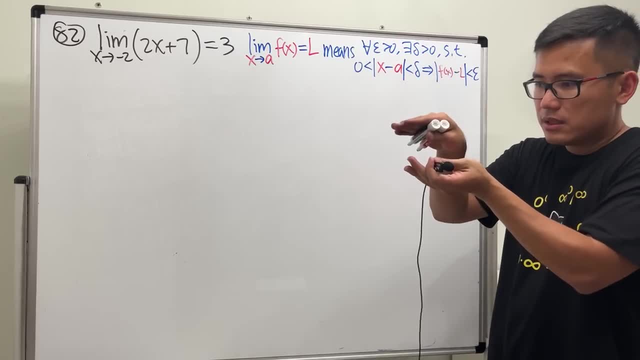 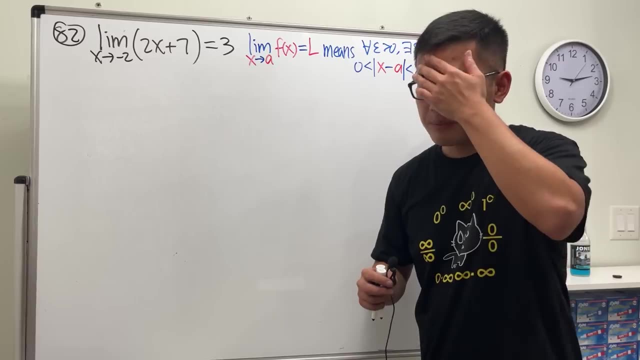 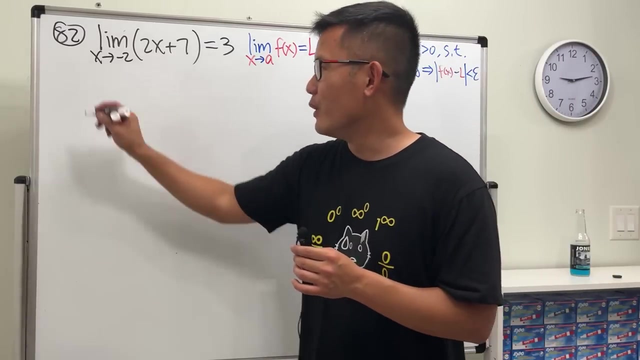 that's why it's E epsilon, It's kind of like it squeeze the, just like kind of make the function as close to the limit as possible, that kind of thing. All right, so now here we go. What's the first thing? 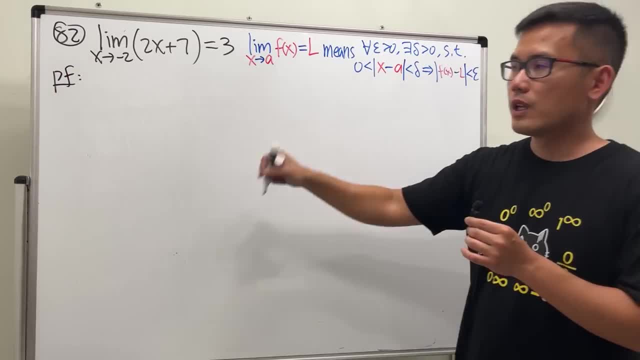 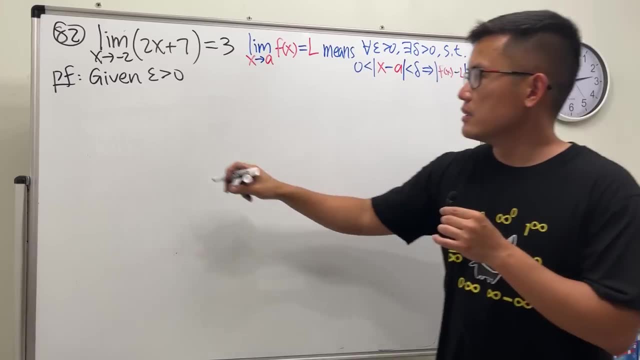 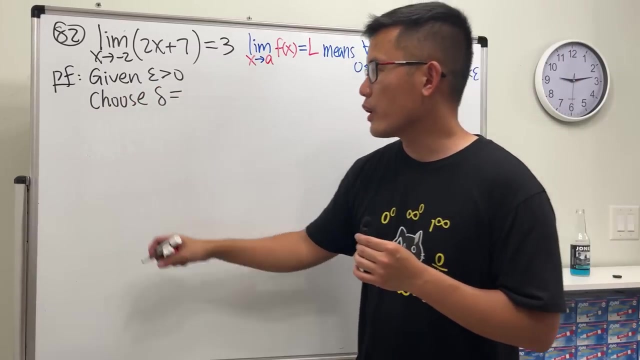 Yes, p, f. Okay for all. go ahead and write down: given epsilon greater than 0. Next, they exist. so we are going to write down: choose delta. delta is what I don't know yet. don't worry, leave it. 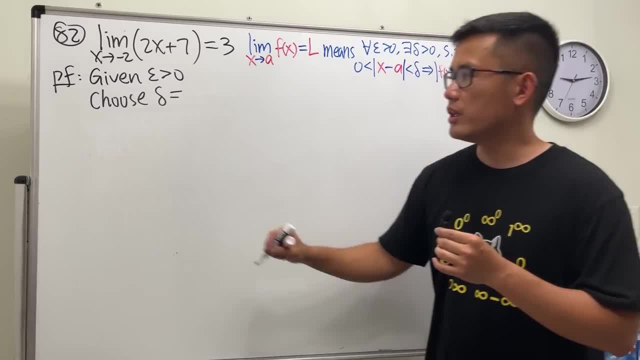 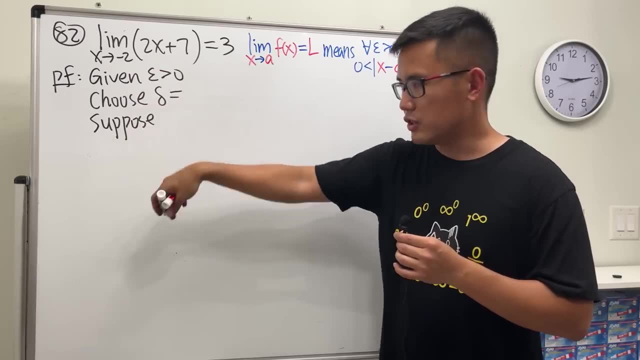 We'll come back to it later. Then we are going to assume we have this condition. So I'm going to suppose, so given suppose, even choose, suppose, and then check, Suppose the absolute value. here we have x. 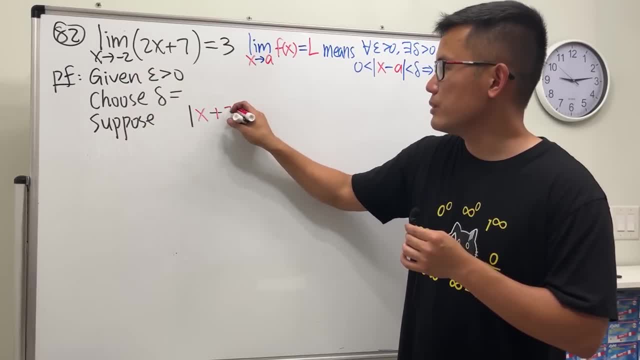 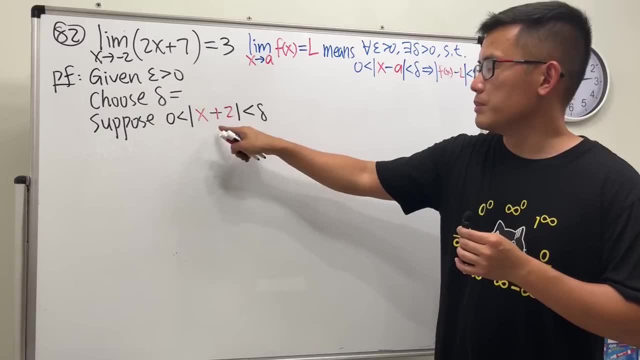 and then minus a, which is negative 2, so it becomes plus 2.. Suppose this right here is less than delta, which we also don't. want x to be negative 2, so that's why you have the greater than 0.. 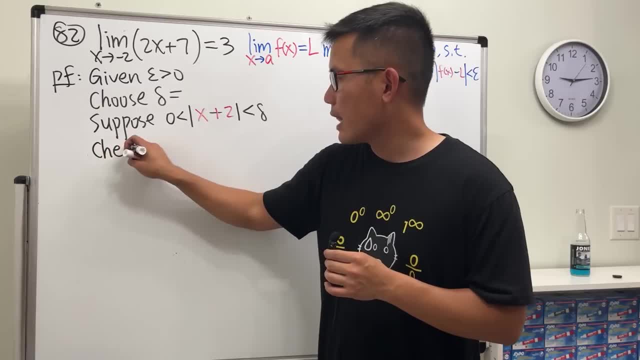 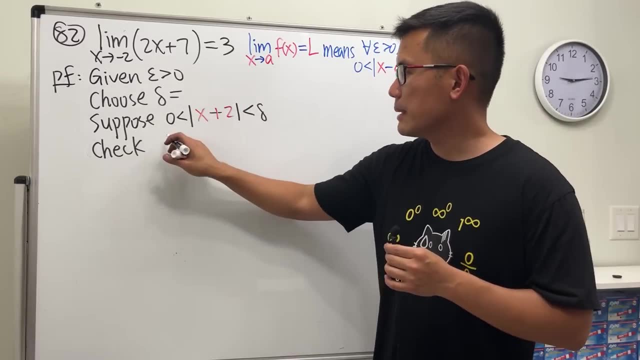 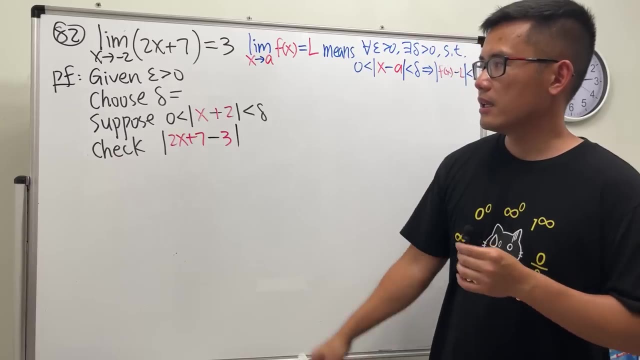 And then check, Check what Absolute value of the function minus the limit, So this minus that, in the absolute value, Two x plus seven and then minus three. All right, Given, choose, suppose, check. Given, choose, suppose check. 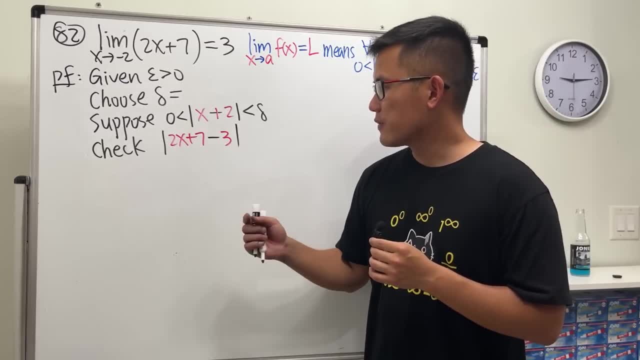 Now focus on this and do the algebra. Seven minus three is four, and then we can actually factor out two. so let's just go and factor that out, it should be okay. So let's just go and factor that out, it should be okay. 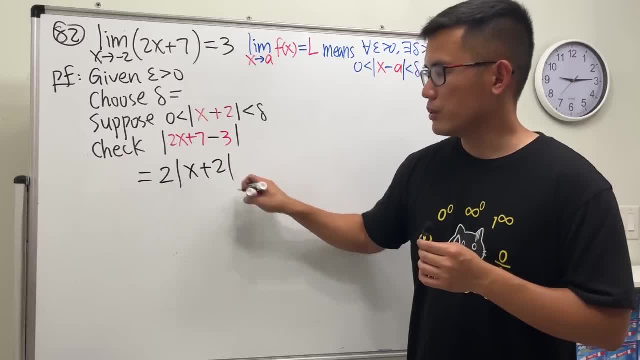 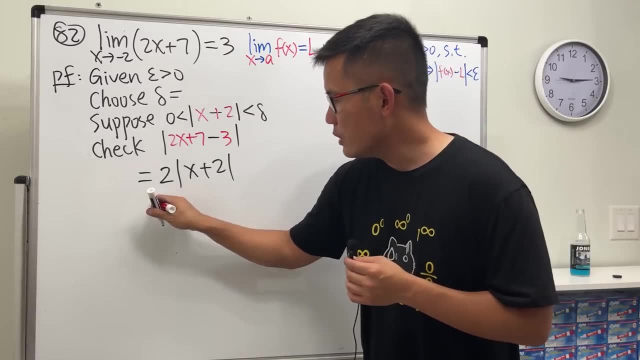 So let's just go and factor that out. it should be okay. And then we end up with what? x plus two, Absolute value of x plus two. so good, because look back this right here we know is less than delta. and then we have a two in the front. 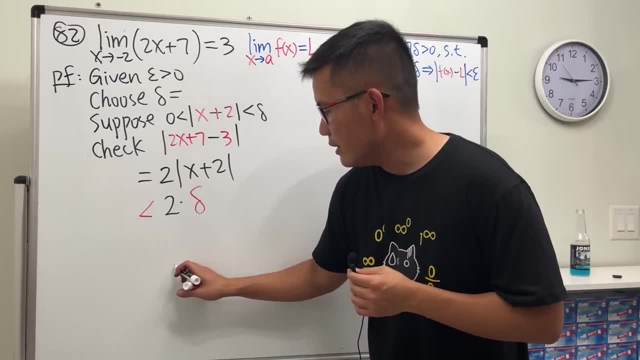 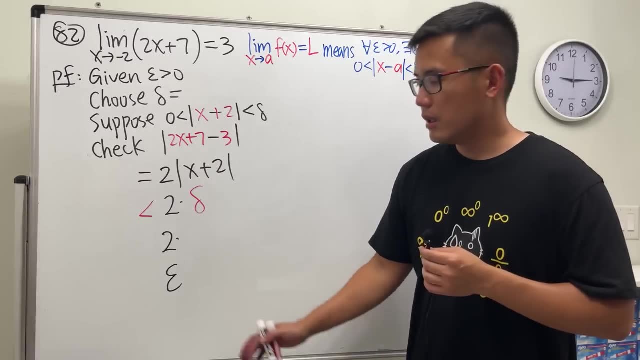 Yeah, Now keep in mind, we want to end up with epsilon. So we have two already. two times four will give us epsilon. We better have epsilon over two, because this way We better have epsilon over two, because this way. 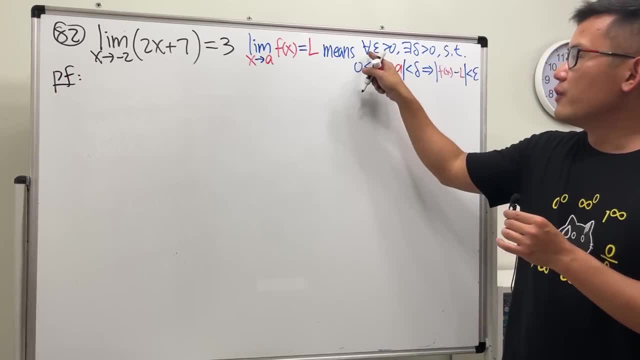 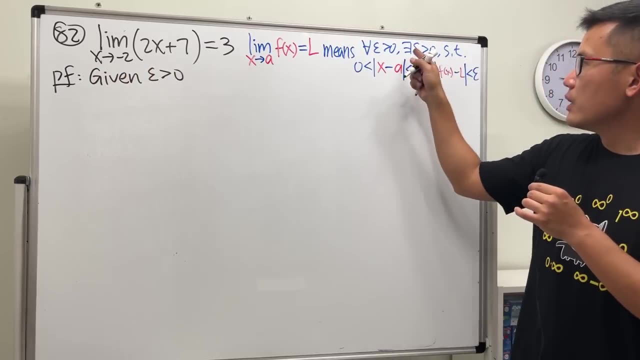 What's the first thing? Yes, p f. Okay for all. go ahead and write down given. Okay For all. go ahead and write down p f- epsilon greater than 0.. Next, they exist, so we are going to write down. 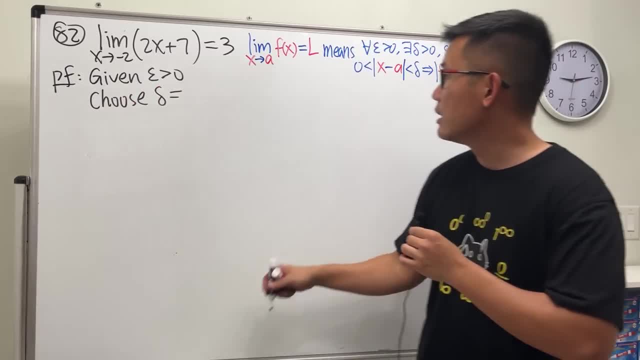 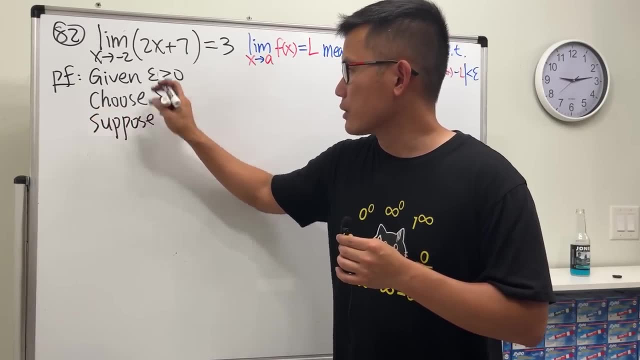 choose delta. delta is what I don't know yet, don't worry, leave it, We'll come back to it later. Then we are going to assume we have this condition, so I'm going to suppose, so given, suppose, even choose, suppose, and then check. 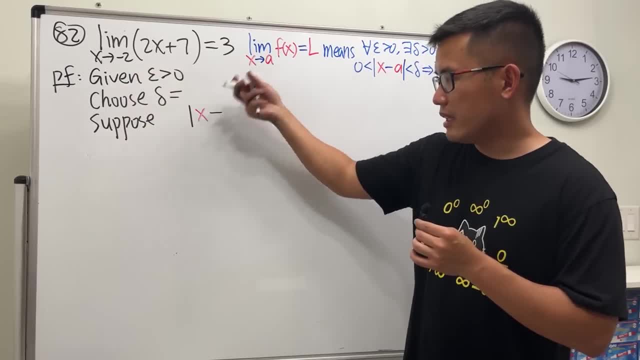 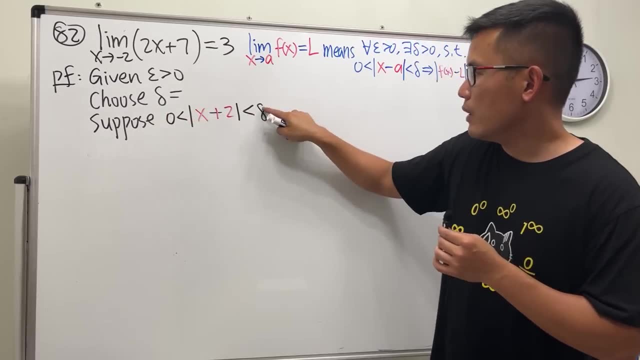 Suppose the absolute value. here we have x and then minus a, so it becomes plus 2.. Suppose this right: here is less than delta, which we also don't. want x to be negative 2, so that's why you have the greater than 0,. 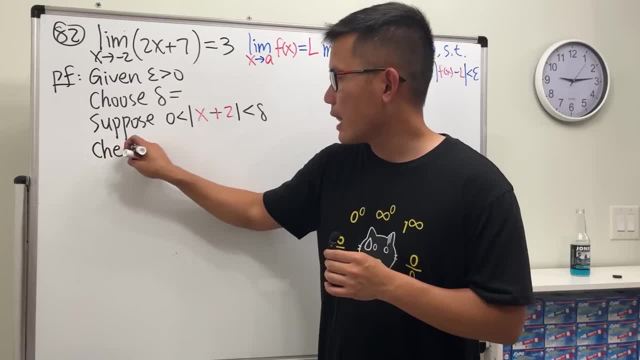 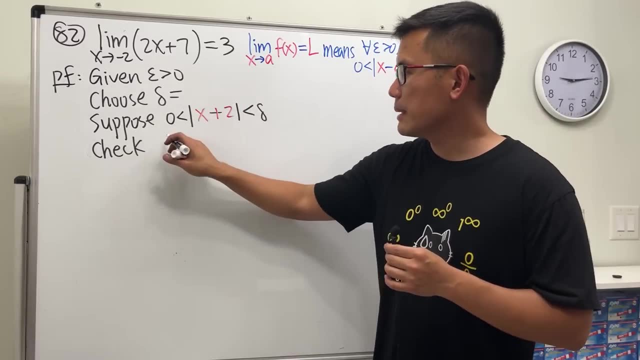 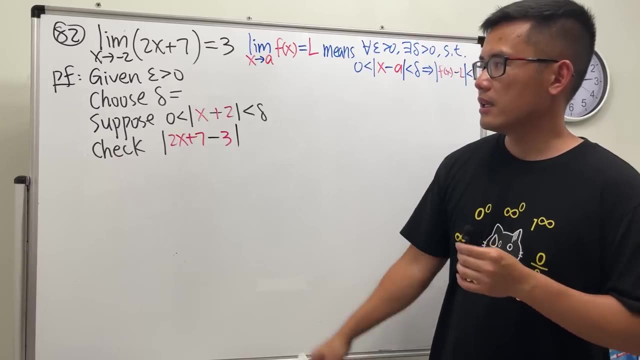 and then check, Check what Absolute value of the function minus the limit. so this minus that in the absolute value 2x plus 7, and then minus 3.. All right, Given, choose, suppose check. Given, choose, suppose check. 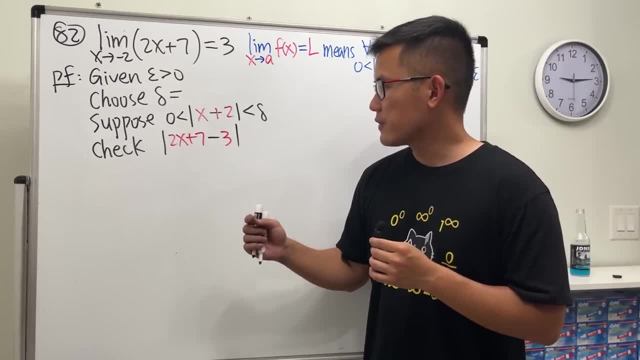 Now focus on this and do the algebra: 7 minus 3 is 4, and then we can actually factor out a 2, so let's just go in and factor that out. it should be okay. and then we end up with what. 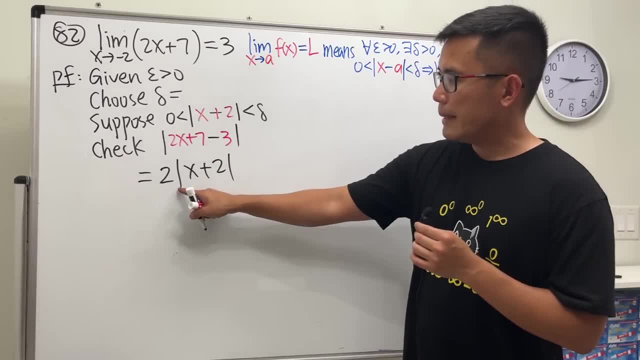 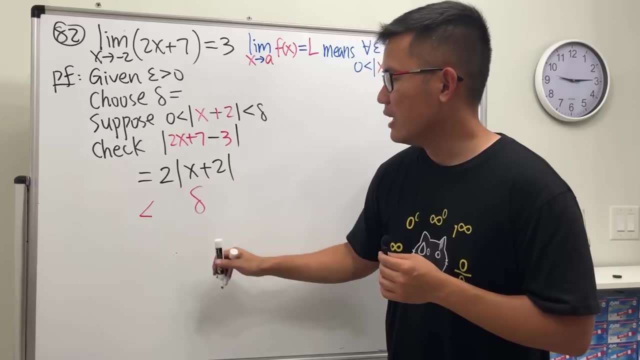 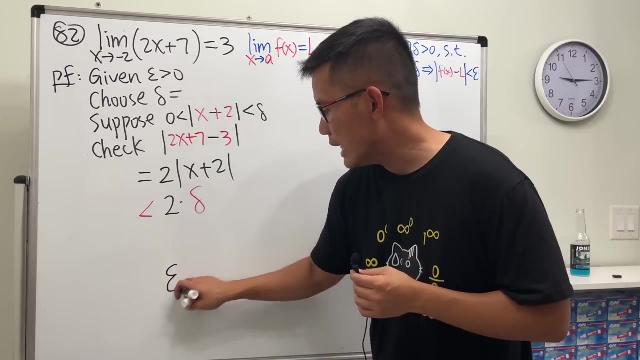 x plus 2.. Absolute value of x plus 2, so good, because look back this right here we know is less than delta, and then we have a 2 in the front. Yeah, Now keep in mind, we want to end up with epsilon. 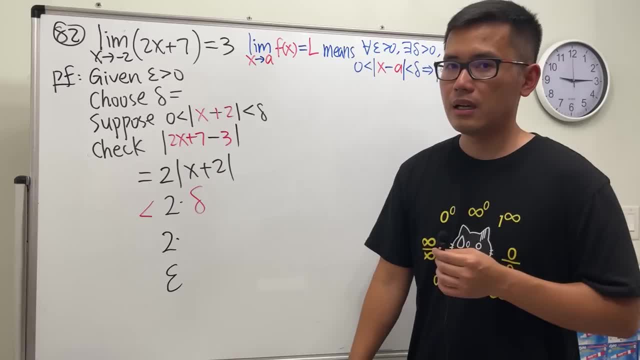 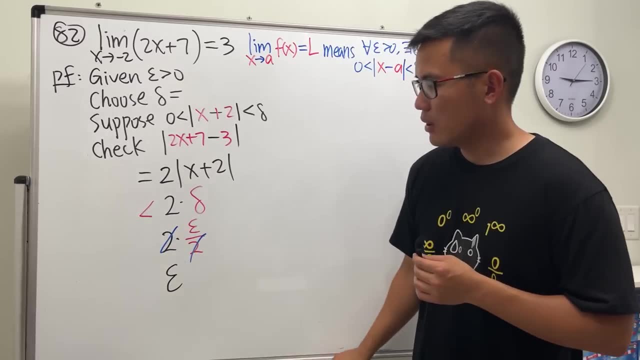 so we have 2 already. 2 times 4 gives us epsilon. We better have epsilon over 2, because this way this 2 and that 2 cancel. so we know we should choose delta to be epsilon over 2.. 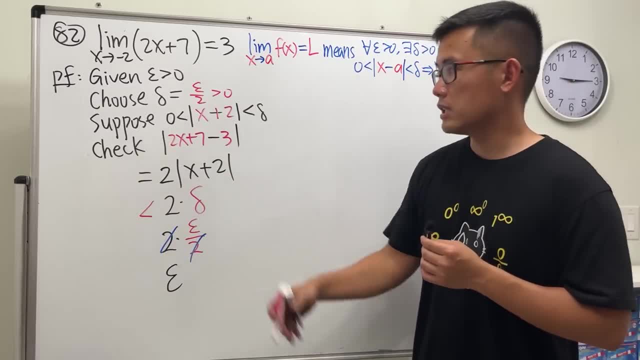 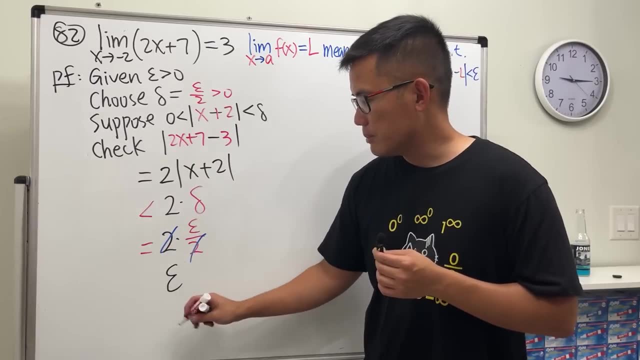 And of course, epsilon is positive over 2 is still positive, so satisfy it. and because delta is epsilon over 2, so we put equal. Likewise. this is just simplification. we put equal sign and we're done. 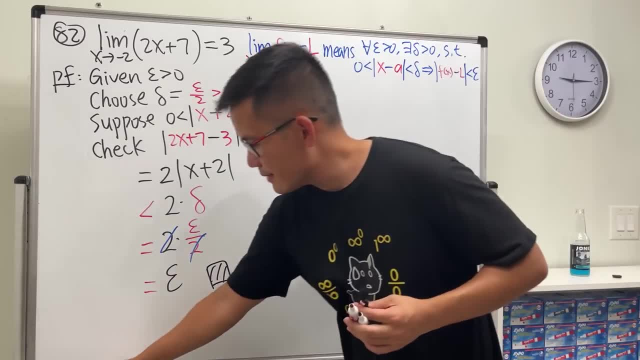 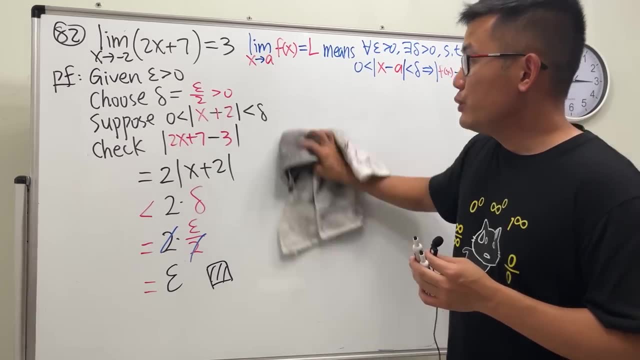 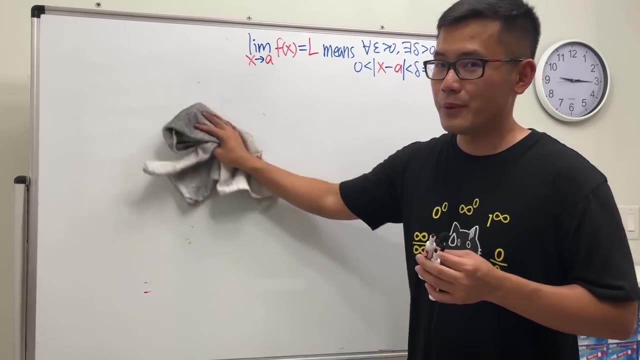 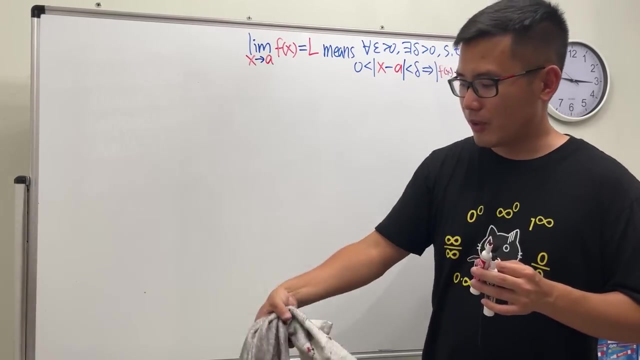 Done Just like that. Okay, Okay, cool, All right, let's do another linear situation. Usually, I'm just saying: usually you will see a linear situation on your exam usually. If not, then a quadratic. Yeah, but I'm going to cover both, so don't worry. 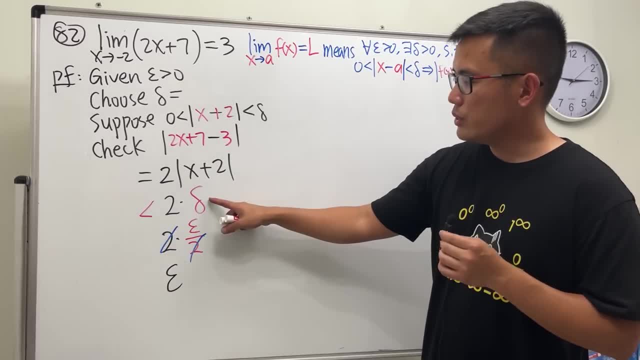 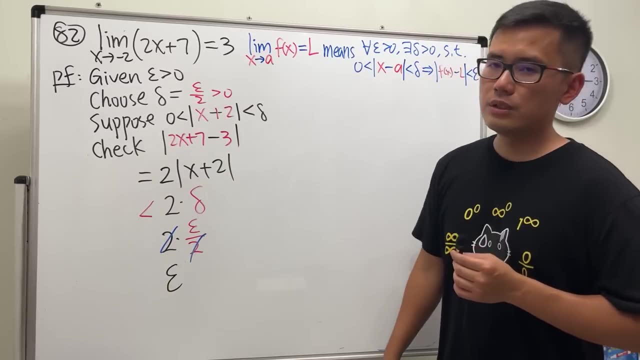 this two and that two cancel. So we know we should choose delta to be epsilon over two. And of course epsilon is positive over two is still positive, so satisfy it. And because delta is epsilon over two, so we put equal. 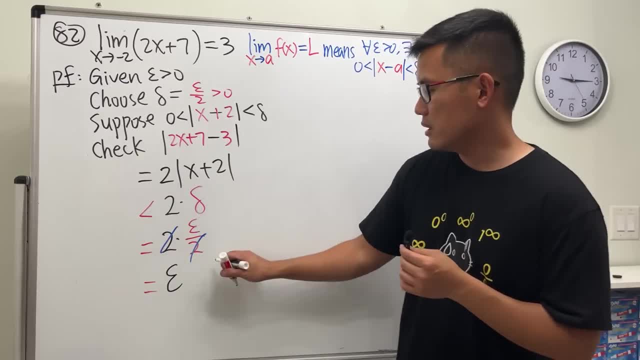 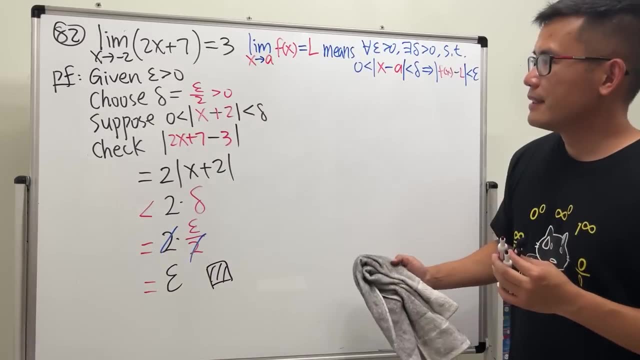 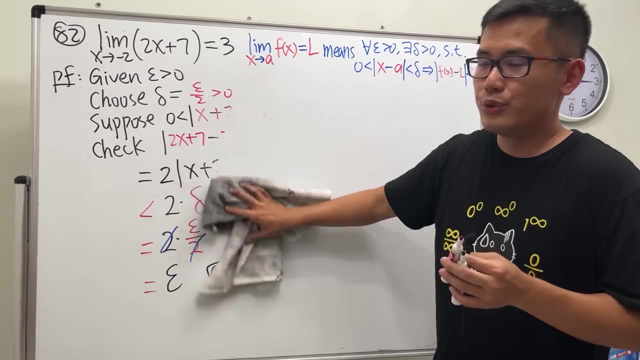 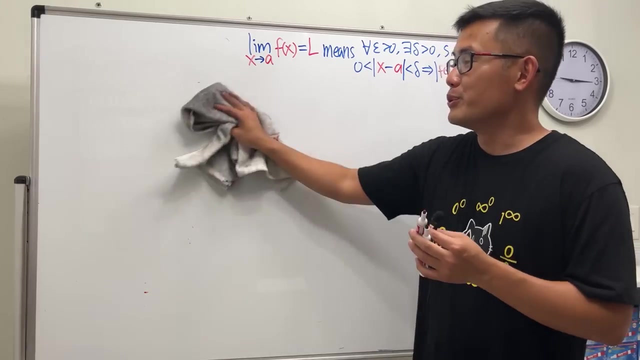 Likewise. this is just simplification. we put equal sign and we're done. Done, just like that, okay, Okay, cool, All right, let's do another linear situation. Usually, I'm just saying usually- you will see a linear situation on your exam usually. 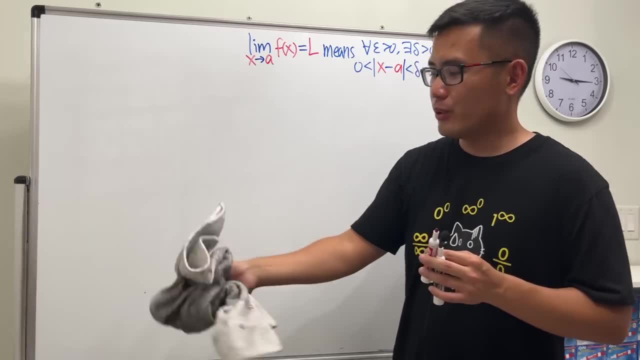 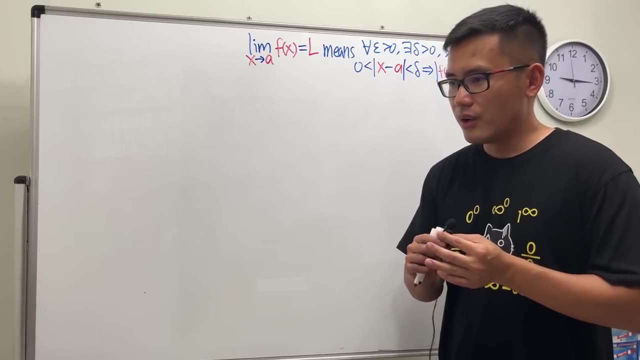 If not, then a quadratic. Yeah, but I'm going to cover both, so don't worry. However, if you are in an honor class, then that's a different story. You might see like a rational or like exponential or like logarithm, but yeah. 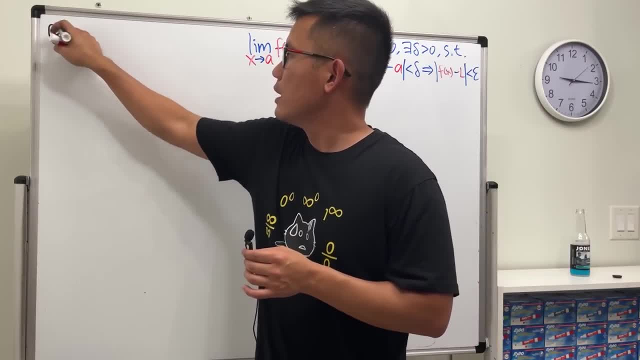 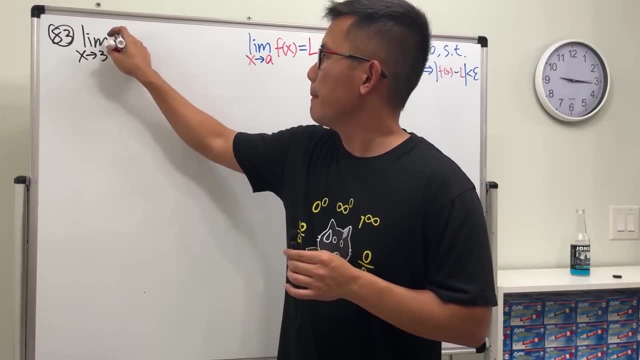 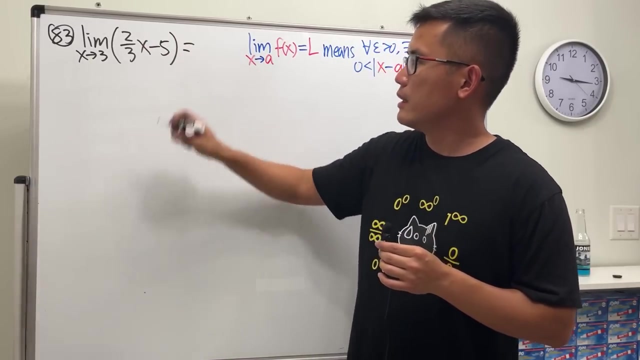 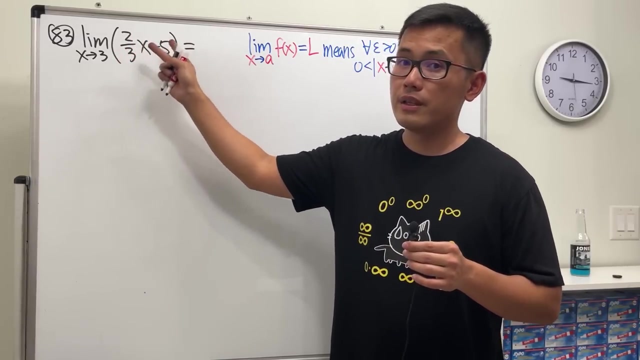 Okay, number 83, limit x approaching three. two over three, x minus five. Okay, let's do this in our head. Put three in here. cancel is two, two minus five. oh, it's a negative three. let me see. 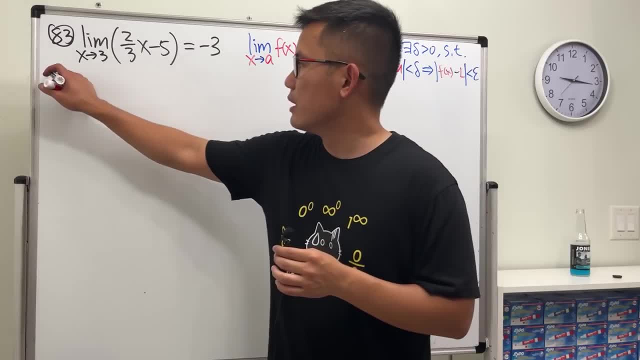 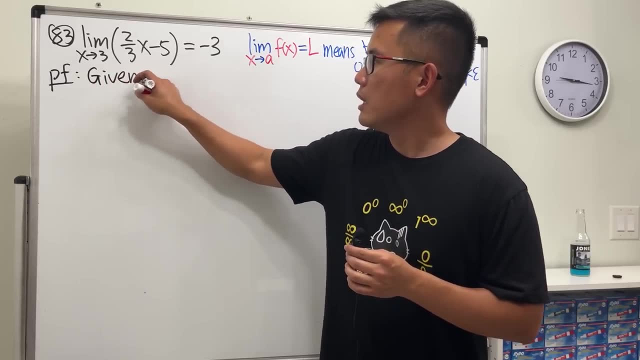 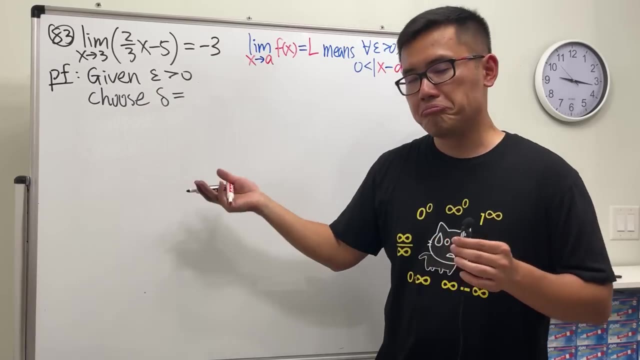 Yeah, okay, cool Here proof: First, given epsilon greater than zero. Next we are going to choose, choose what. Choose delta to be what Don't know. leave it Then, suppose, suppose, the distance between x and three. 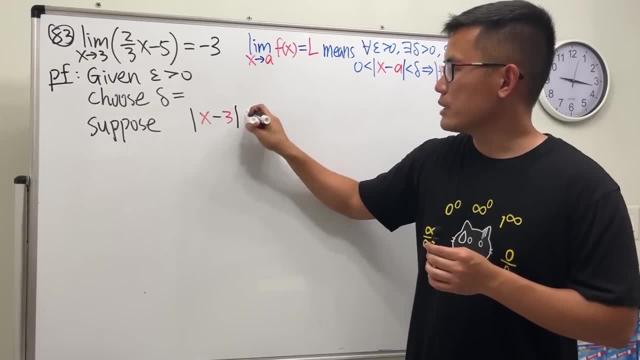 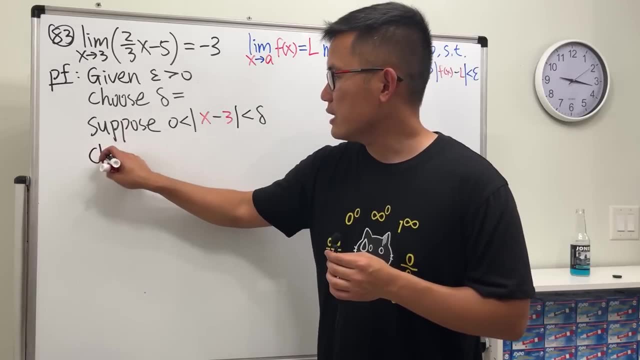 so we say x minus three. we want this to be less than delta, so we don't want x to be three. so put a greater than zero. looking it backwards, then we check Absent value of the function minus the limit. 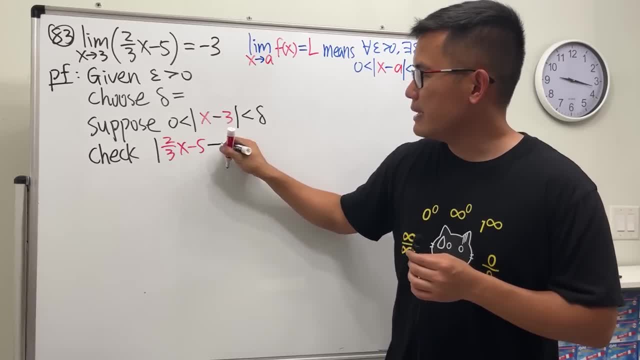 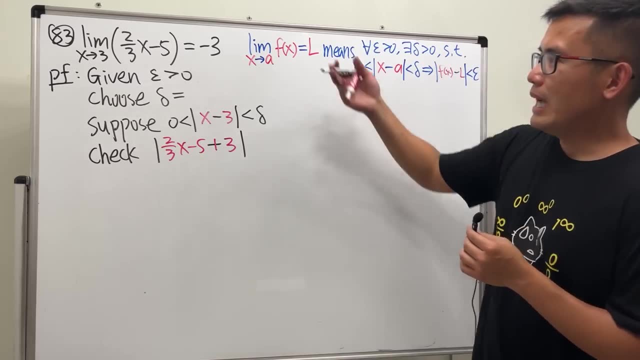 So we are looking at two over three, x minus five minus negative three, so it becomes plus three. Okay, here we go. We have a fraction. so that's how it goes. Okay, negative five plus three is negative two. so here we have. 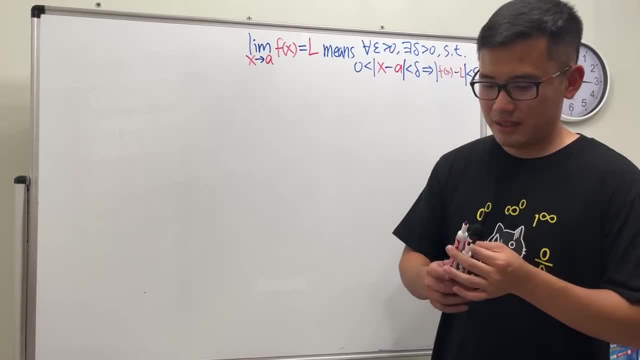 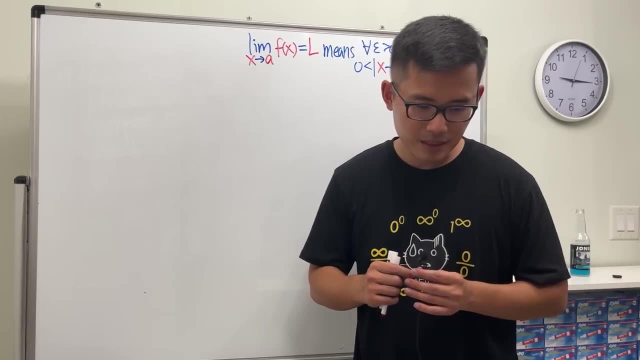 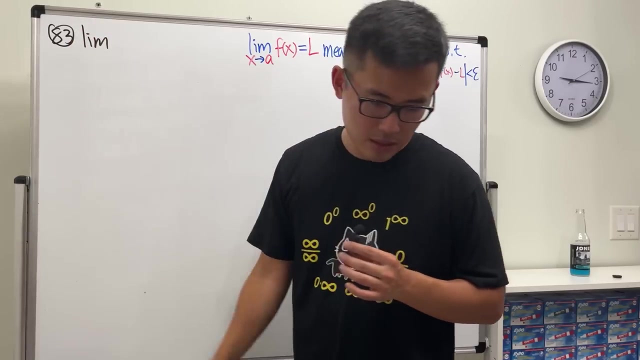 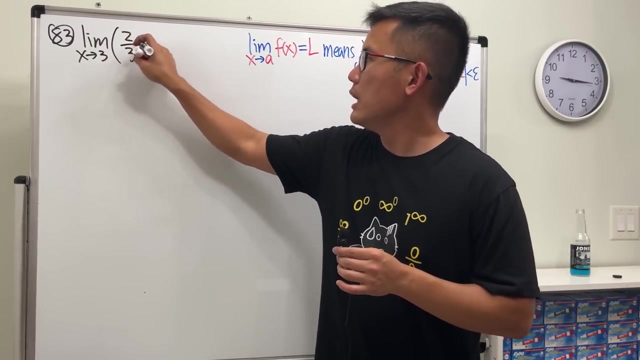 However, if you are in an honor class, then that's a different story. You might see like a rational or like exponential or like logarithm. But yeah, Okay, number 83.. Limit x approaches 3, 2 over 3, x. 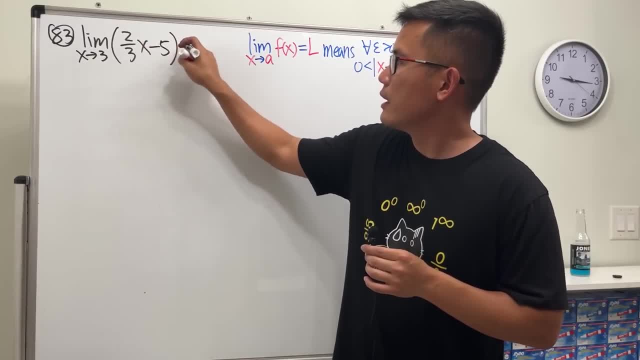 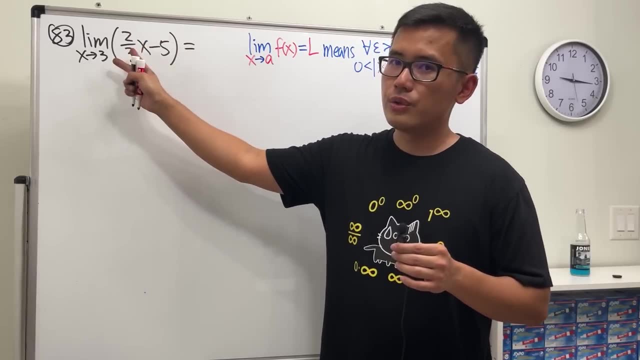 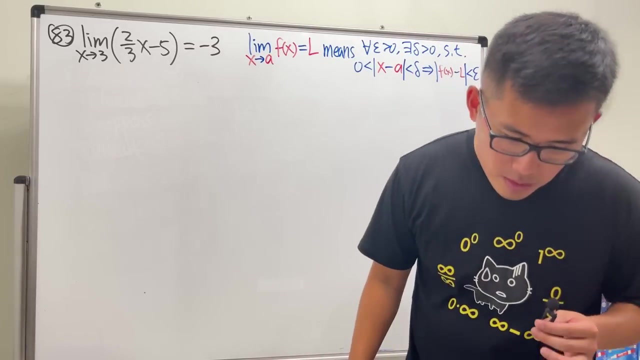 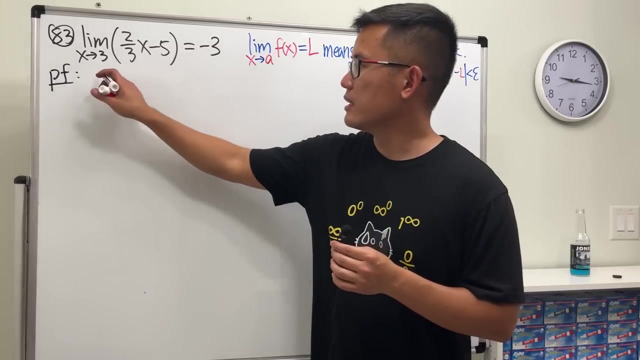 minus 5.. Okay, let's do this in your head. Put 3 in here. Cancel is 2, 2 minus 5 is a negative 3.. Let me see, Yeah, okay, cool Here. proof First, given epsilon greater than 0.. 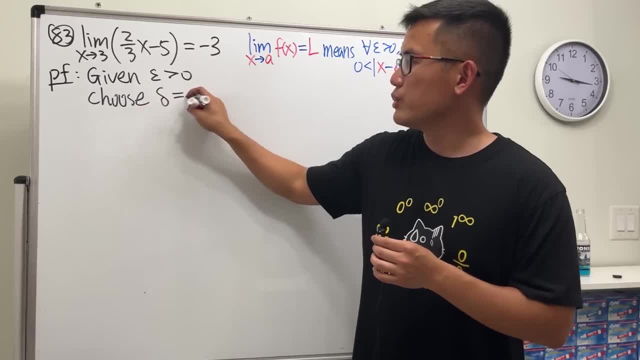 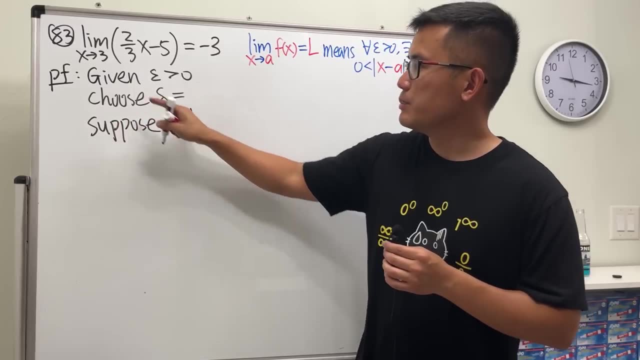 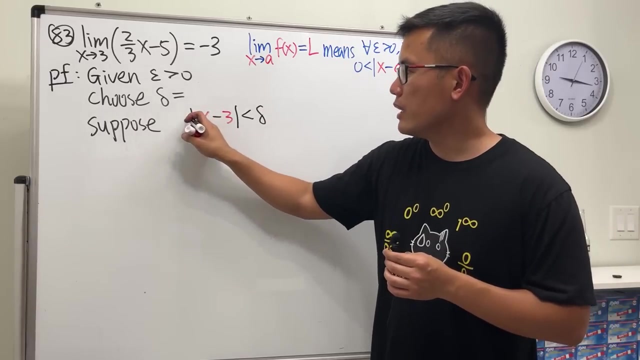 Next, we are going to choose what. Choose delta to be what Don't know. Leave it Then. suppose the distance between x and 3. So we say x minus 3. We want this to be less than delta and we don't want x to be 3.. 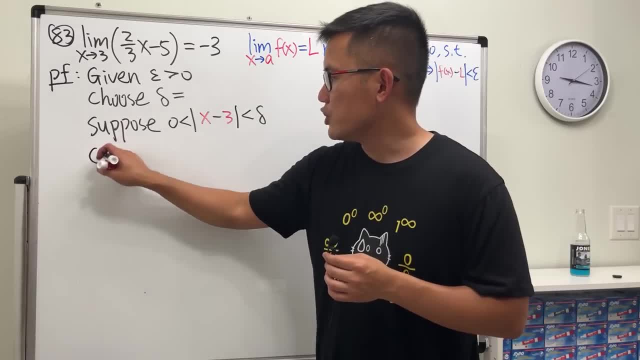 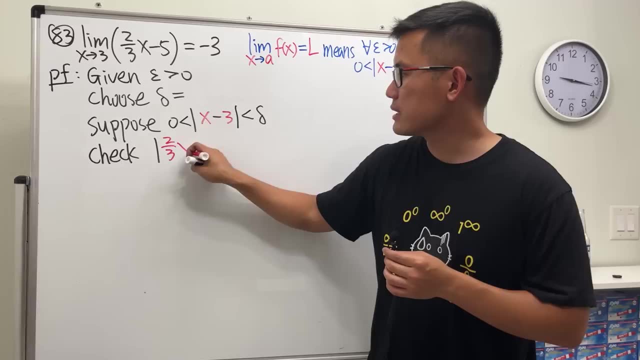 So put a greater than 0.. Looking backwards then we check absolute value of the function minus the limit. So we are looking at 2 over 3x, minus 5,, minus 3.. Negative 3, so it becomes plus 3.. 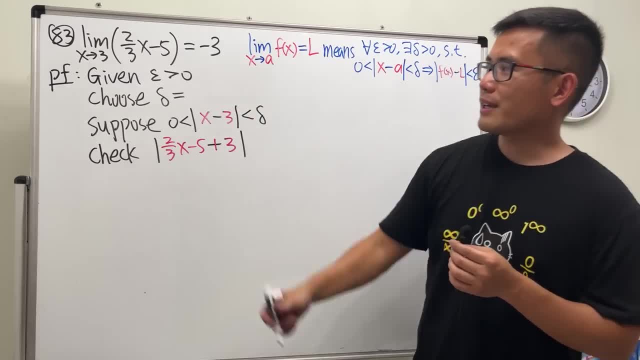 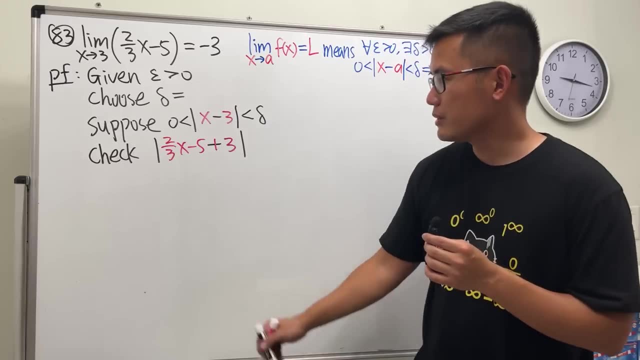 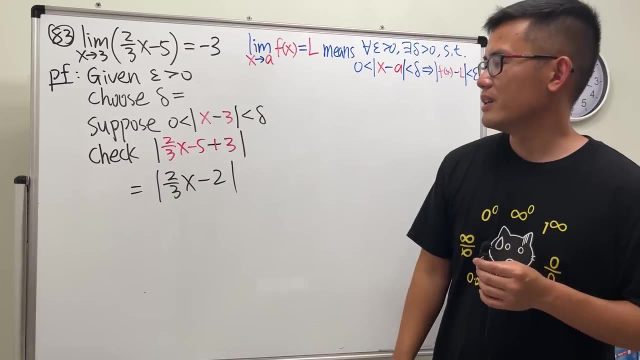 Okay, here we go. We have a fraction, so let's see how it goes. Okay, negative 5 plus 3 is negative 2.. So here we have 2 over 3x minus 2.. Okay, Can we factor it? Yes? 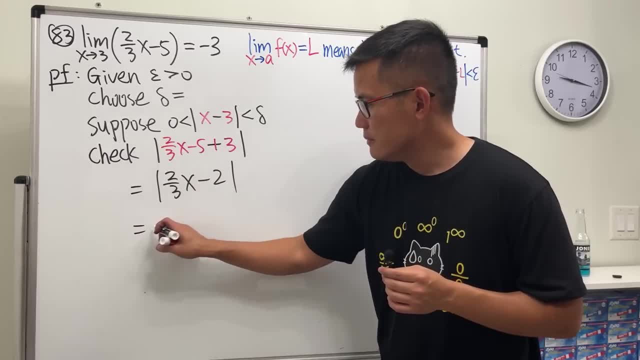 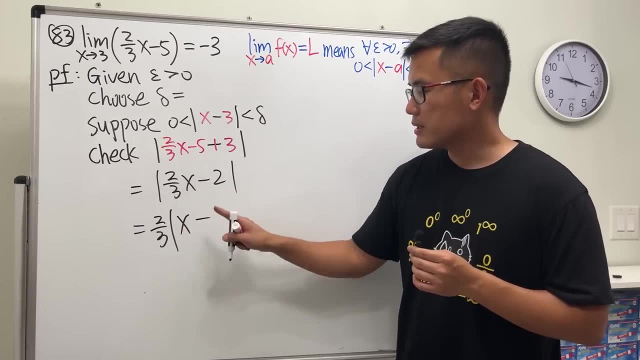 We can still factor out the 2 over 3.. Check this out, So I break this up: So it's x and then we have the minus, But originally here is minus 2. We factor out the 2 over 3.. 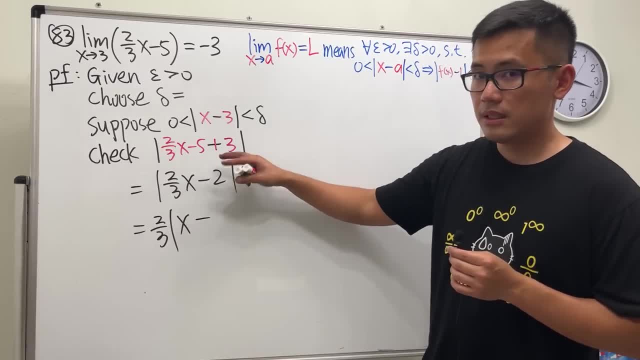 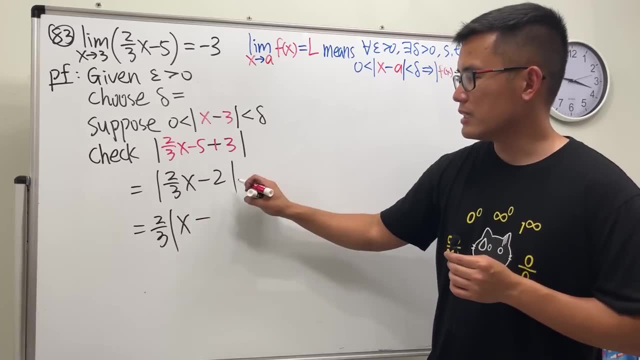 So what should we do? We should look at this and divide it by. we should just look at this: divided by that, Divided by 2 over 3, is the same as multiplied by 3 over 2.. They cancel, so we just have just a 3.. 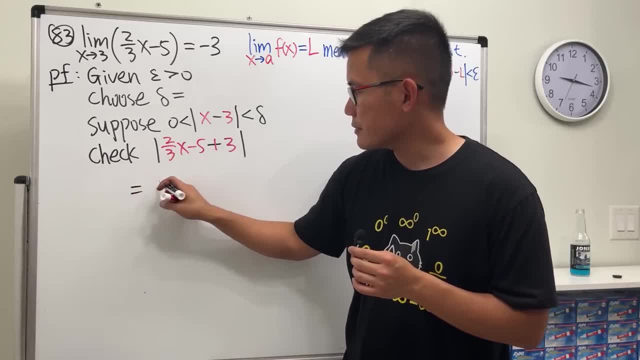 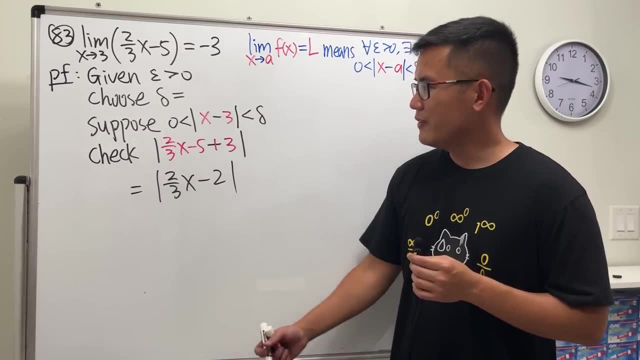 negative. five plus three is negative two. so here we have negative three is negative two. so here we have: We have 2 over 3, x minus 2.. Okay, Can we factor it? Yes, We can still factor out the 2 over 3.. 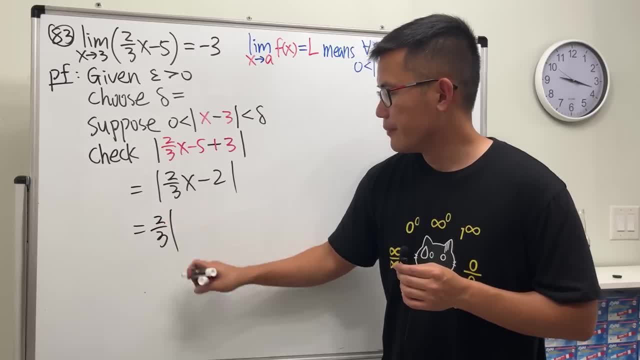 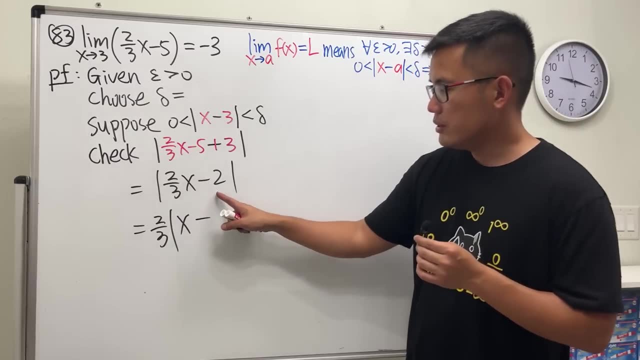 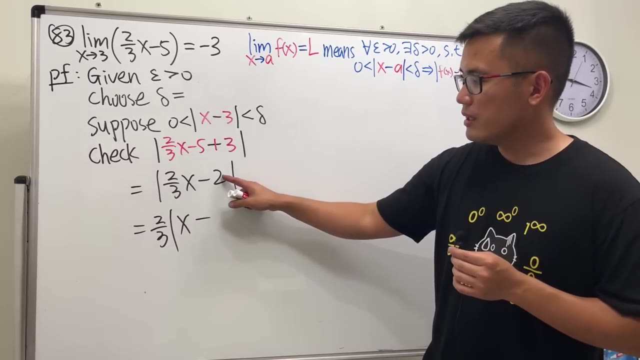 Check this out. So I break this up. so it's x And then we have the minus, But originally here is minus 2. We factor out the 2 over 3.. So what should we do? We should look at this and divide it by. 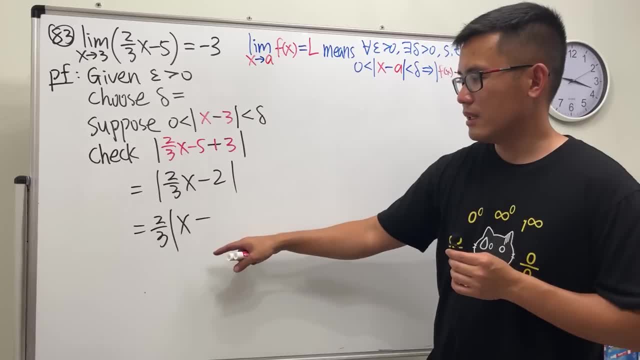 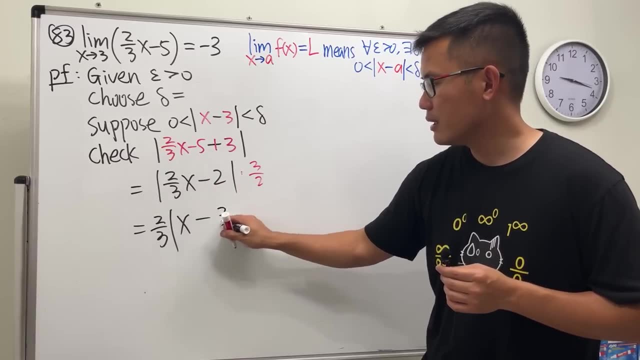 We should just look at this. divide it by that. Divide it by 2 over 3 is the same as multiply by 3 over 2.. They cancel, so we just have just a 3.. I'm not kidding, Check this out. 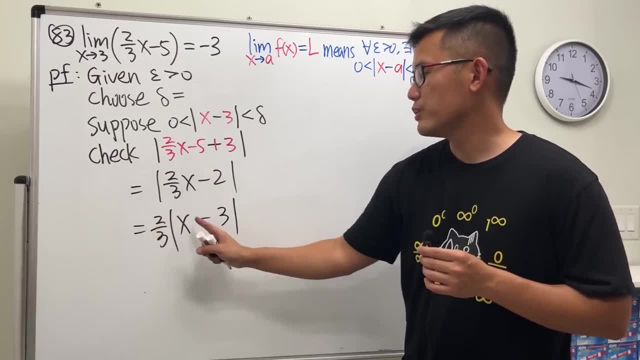 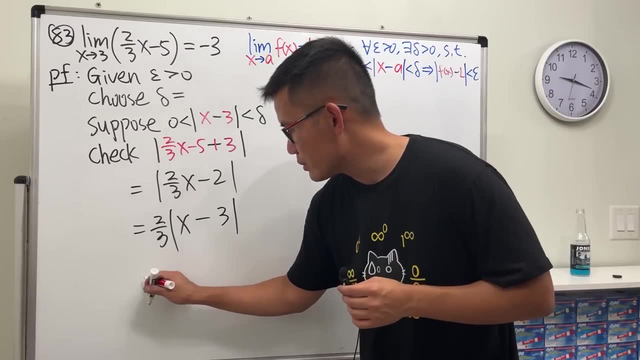 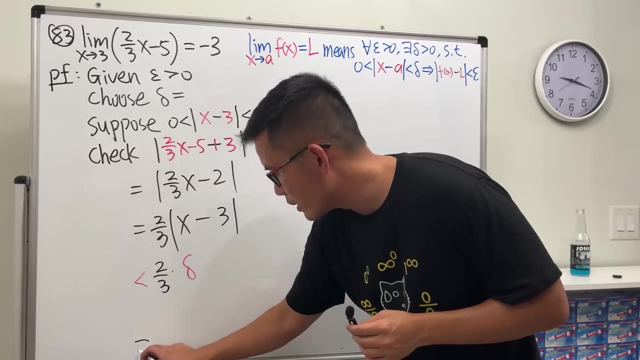 Distribute it back. we get this This times that 3 cancels 2 minus. Yeah, What's this Less than delta? So we know this right here. This is 2 over 3 times delta And at the end, we want this to be equal to epsilon, right? 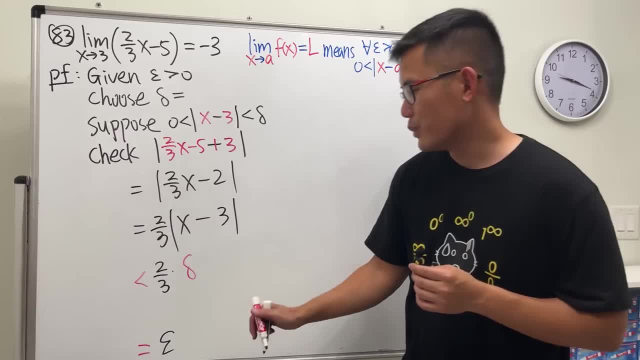 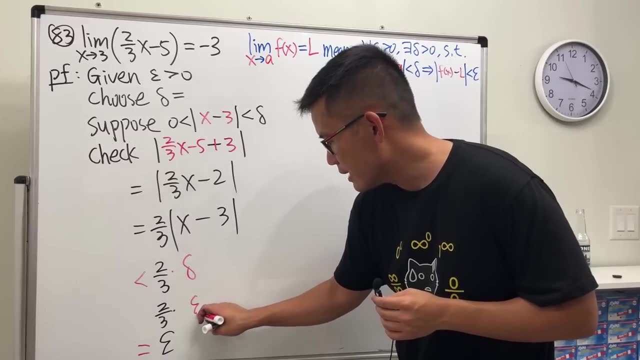 So you know it, Delta shall be equal to what? Well, this right. here we will have to kind of work it out a little bit. 3 over 2 times: Okay, You want to have epsilon here, And then perhaps we just need a reciprocal right. 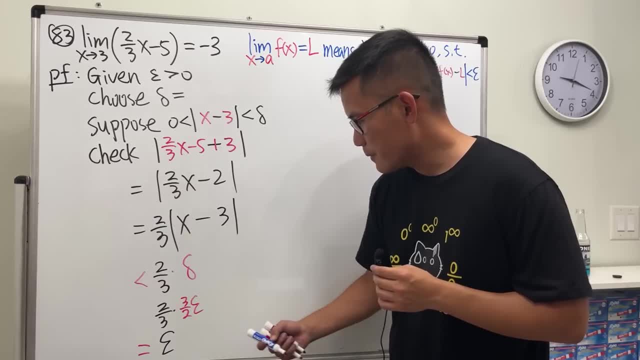 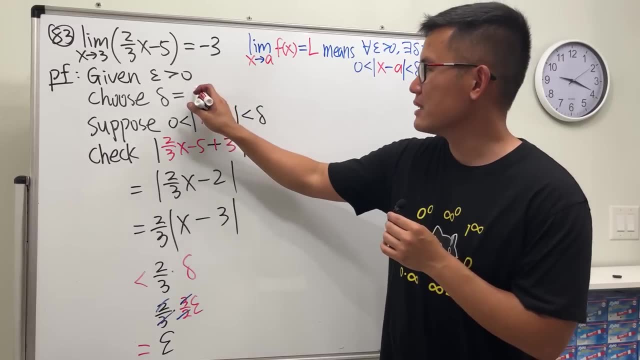 Namely 3 over 2. Because this way 2 and 2. Cancels 3 and 3 cancel Perfect. So that means delta is equal to 3 over 2 epsilon. Yeah, This is equal to that. 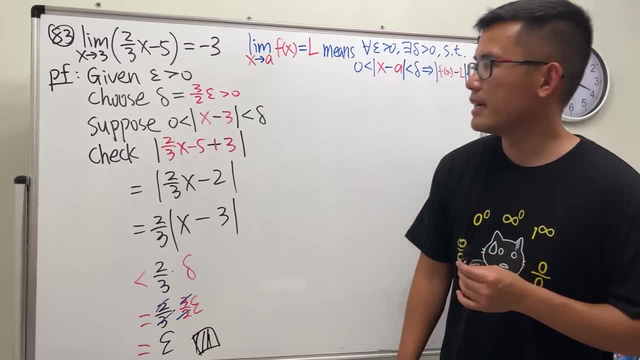 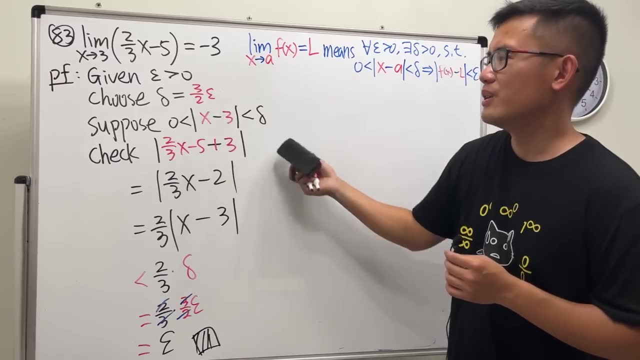 Put it there, Done, Yeah, And, as I said, you don't necessarily need to put a greater than 0.. This is okay, Yeah, Because in my previous video I don't think I put down like delta is this and a greater than 0.. 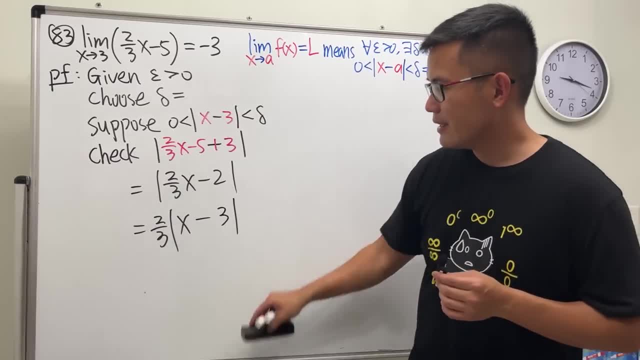 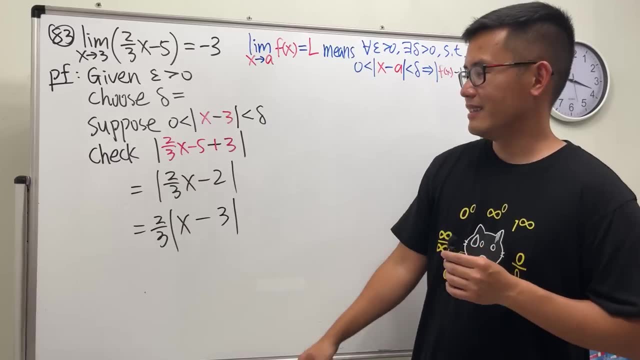 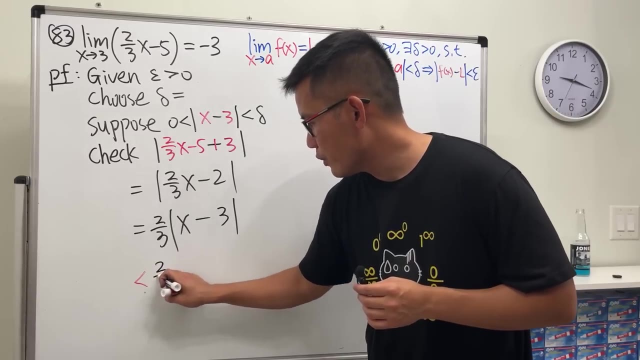 I'm not kidding. Check this out, Distribute it back. we get this This times that 3 cancels 2 minus. Yeah, What's this Less than delta? So we know this right here is 2 over 3 times delta. 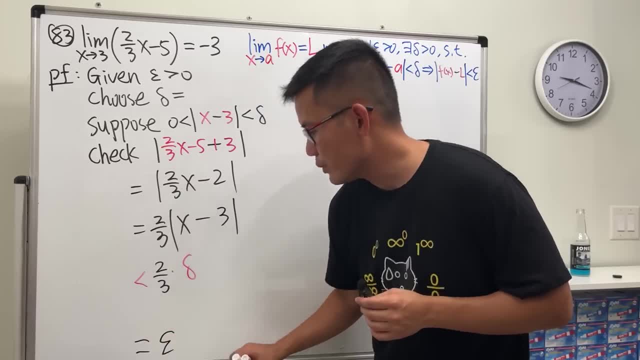 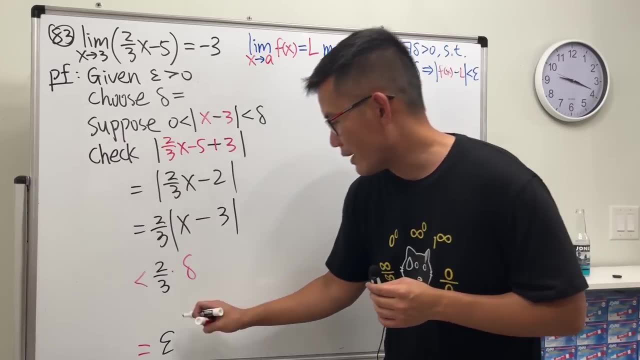 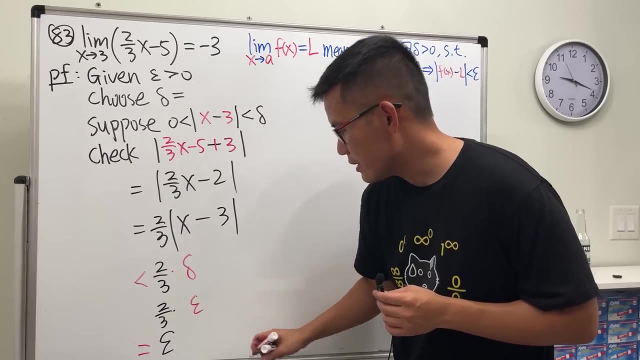 And at the end we want this to be equal to epsilon, right? So you know it, Delta shall be equal to what? Well, this right here we will have to kind of work it out a little bit. 3 over 2 times. OK, you want to have a epsilon here? 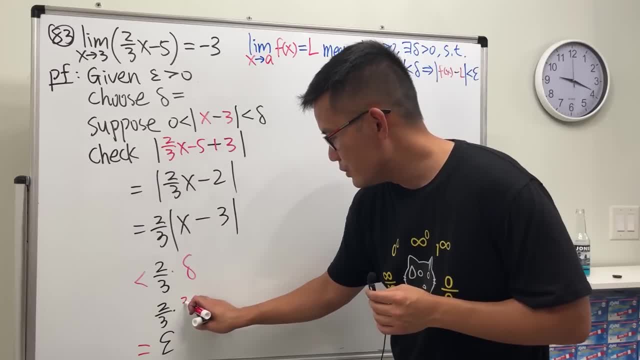 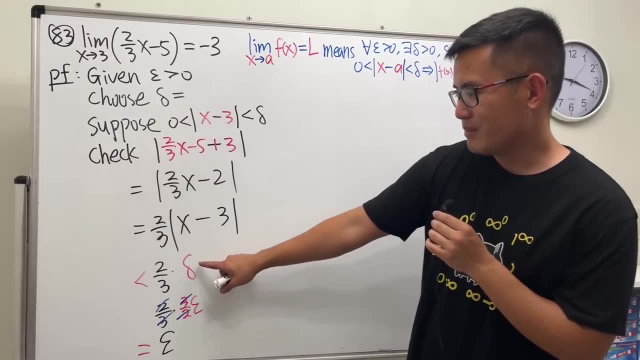 And then perhaps we just need a reciprocal right, Namely 3 over 2, because this way 2 and 2 cancel 3 and 3 cancel, perfect. So that means delta is equal to 3 over 2 epsilon. 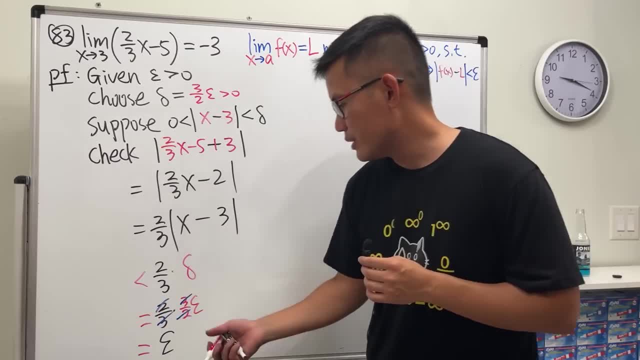 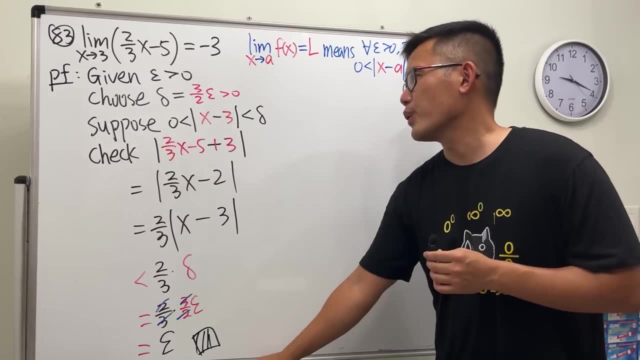 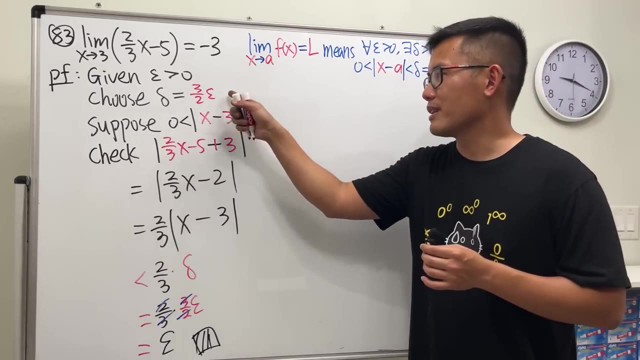 Yeah, This is equal to that. put it there, done. Yeah, And, as I said, you don't necessarily need to put a greater than 0.. This is OK, Yeah, Because in my previous video I don't think I put down like delta is this and a greater than 0.. 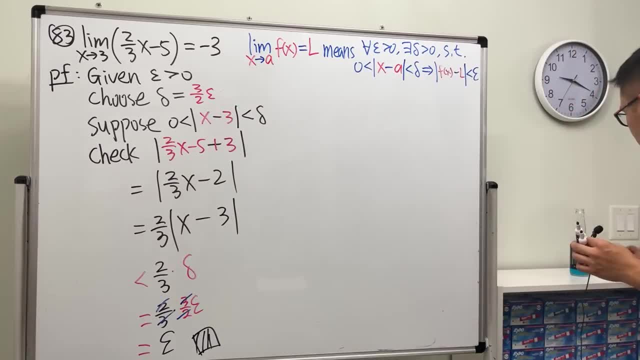 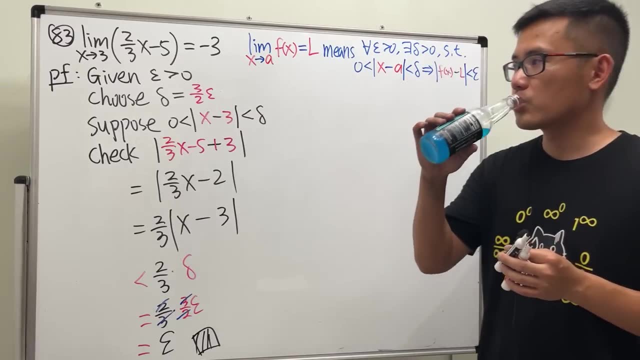 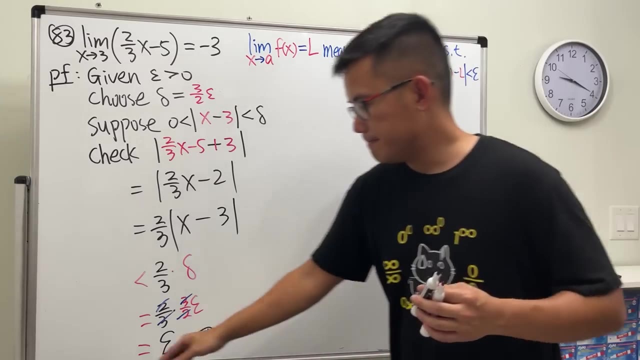 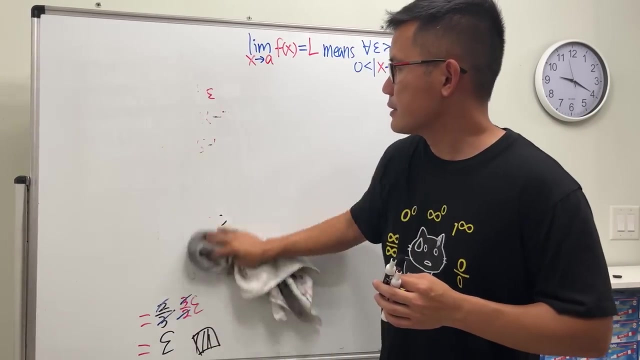 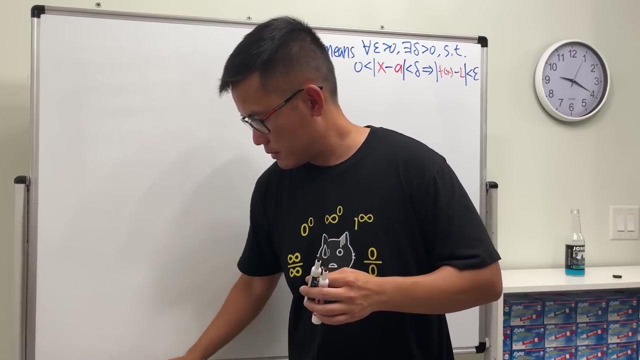 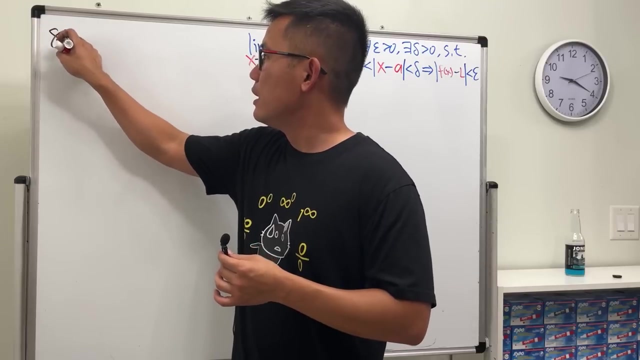 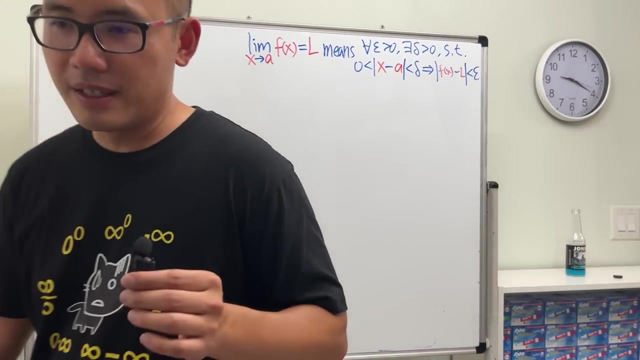 Usually you can just write down formula and that's it. So here are the three examples for epsilon-delta definition. when the function is linear, All right, number 84, let's look at a first situation that the function is not linear. And then why don't I look at the? OK, it's. 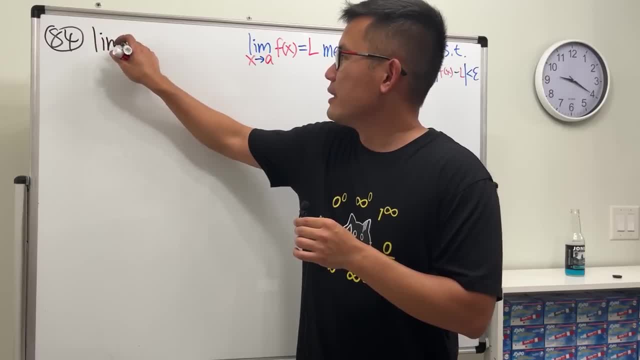 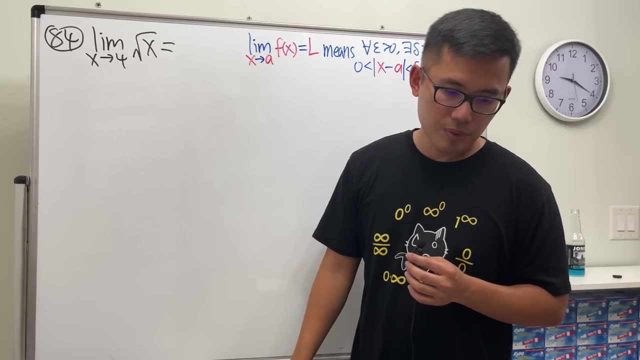 it's, it's, it's, it's going all right. Anyway, take a limit as x approaching 4, and then we have the square root of x. Man this, if it's a computational question, it's super easy, because the answer is just 2.. 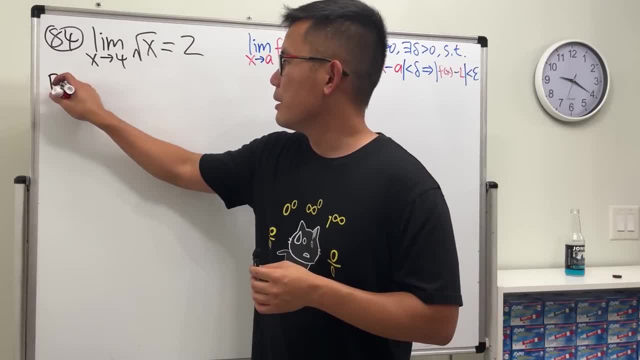 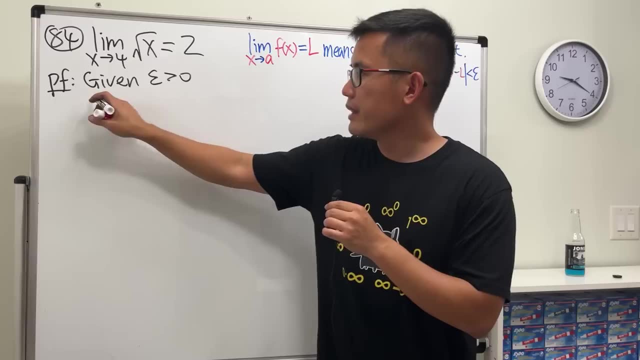 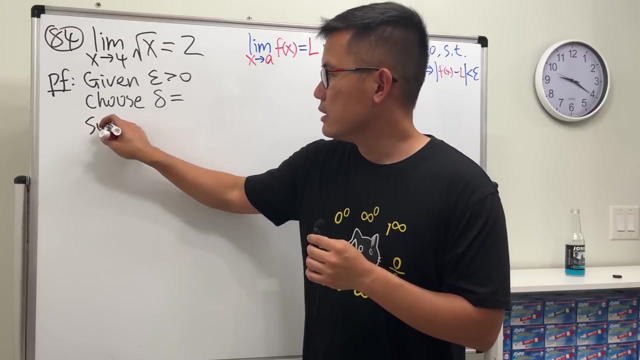 Yeah, but for proof let's just go ahead and do it. P, F, here we go, given epsilon greater than 0.. Next we are going to choose delta. I don't know. just leave it Then, suppose. 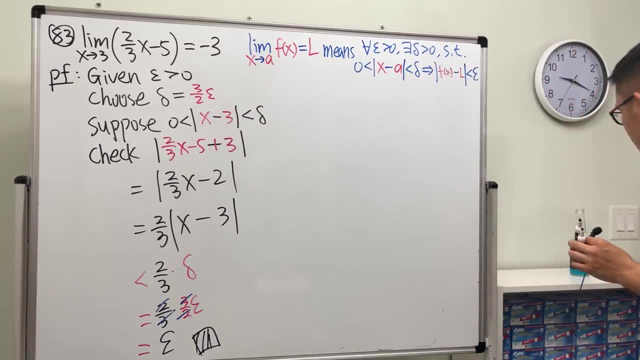 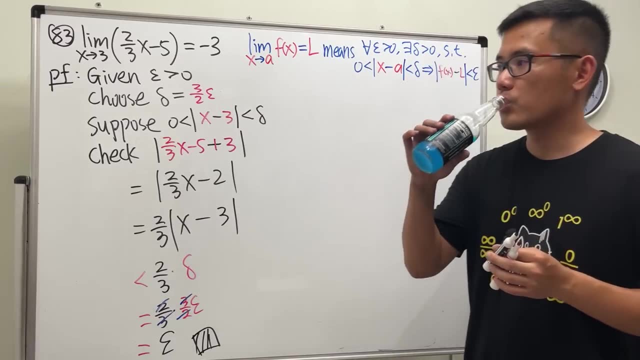 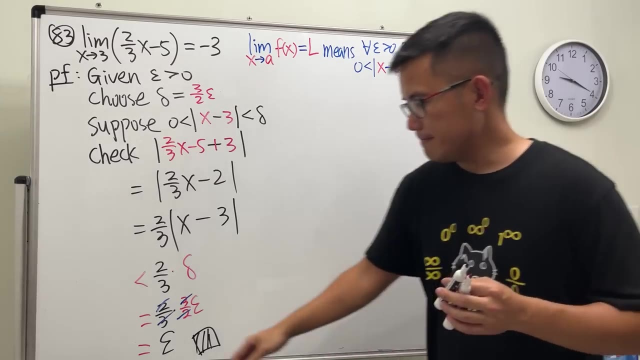 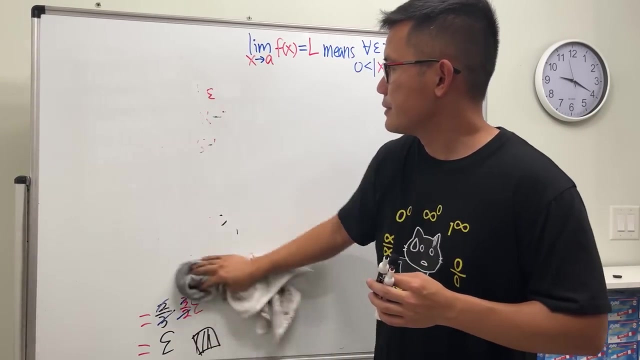 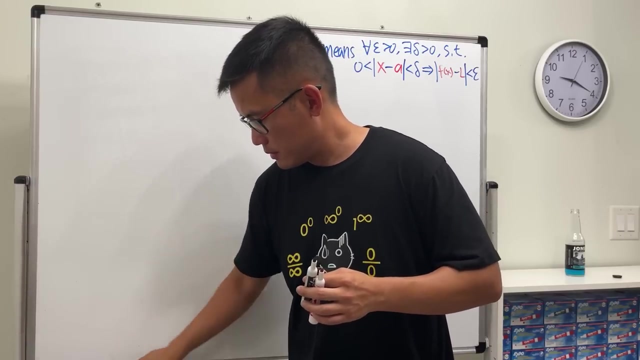 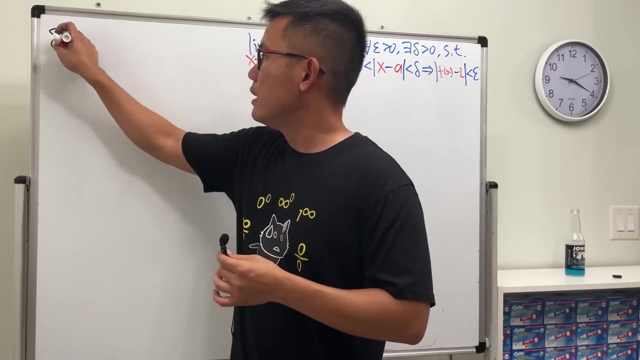 Usually you can just write down 4. And that's it. So here are the three examples for epsilon-delta definition when the function is linear. Thank you, See you in the next video, Bye-bye, Bye-bye. 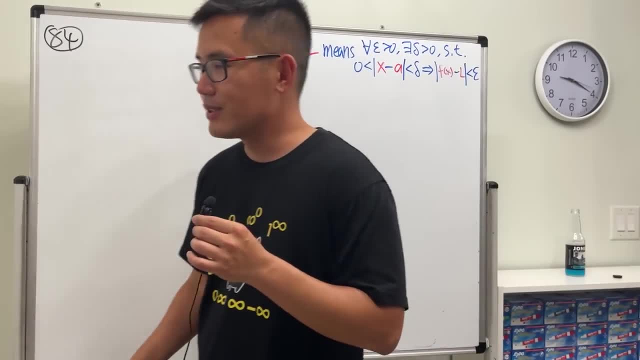 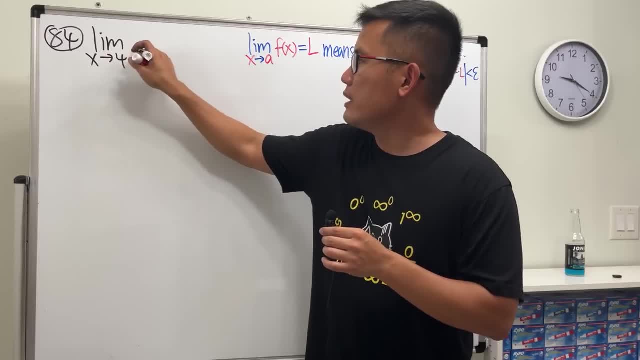 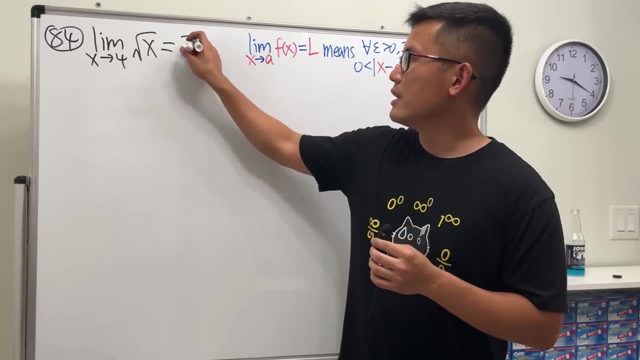 Anyway, Take a limit as x approaching 4, and then we have the square root of x. Man. this, if it's a computational question, is super easy. huh, Because the answer is just 2.. Yeah, But for proof let's just go ahead. 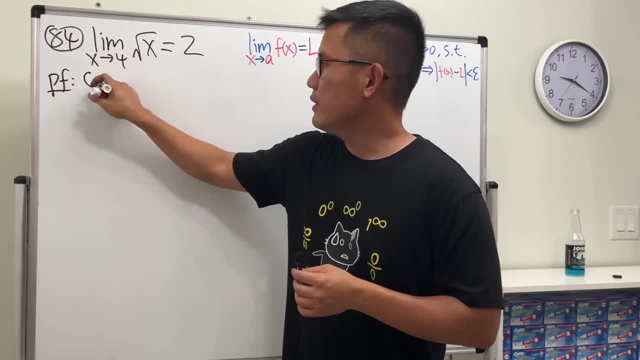 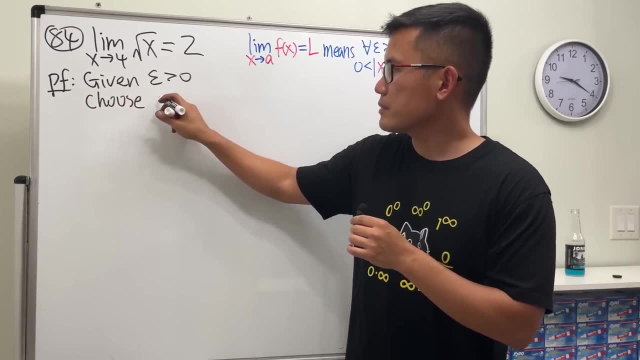 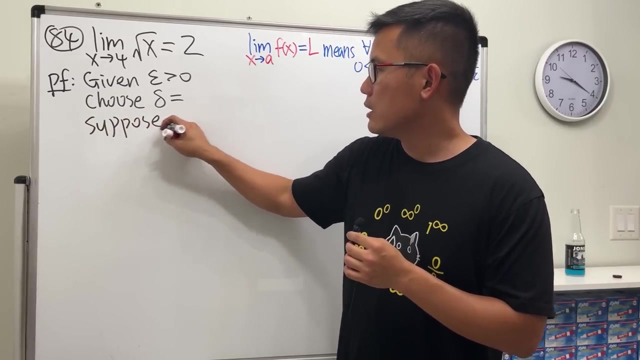 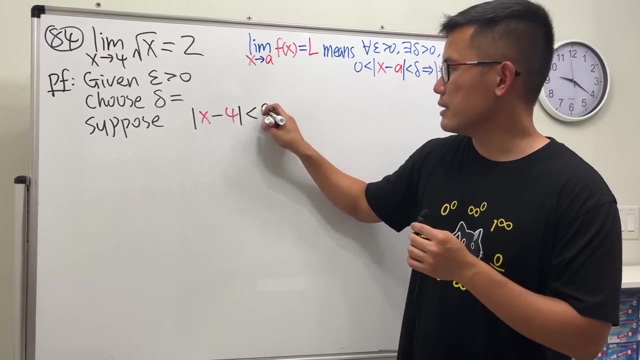 it p, f. here we go, given epsilon greater than zero, next we are going to choose delta. i don't know. just leave it then suppose, suppose what absolute value of x minus 4 to be less than delta and then greater than zero. we'll get backwards. and then, lastly, we check. 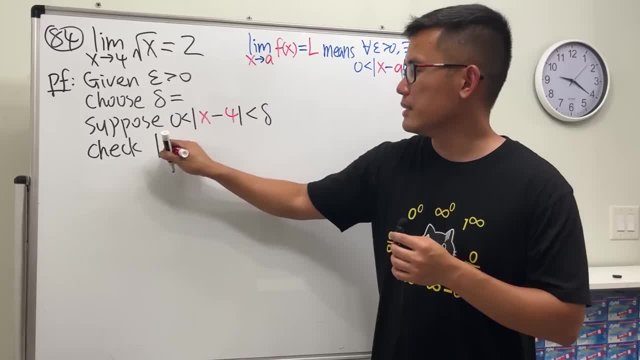 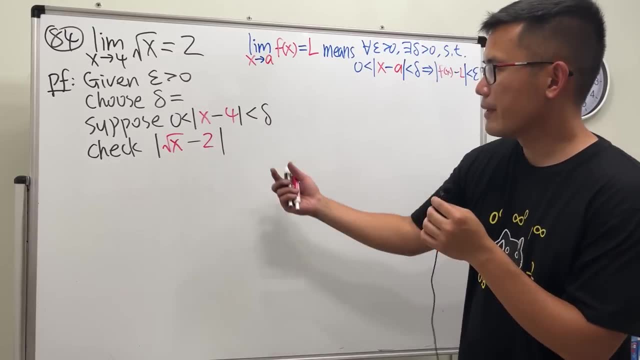 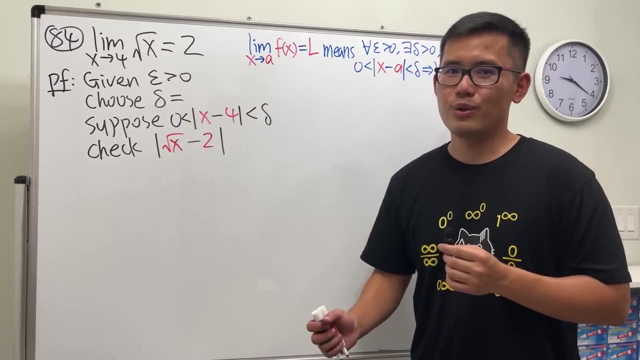 absolute value function minus the limit. okay, that's all you have all. right now we cannot factor this anymore, huh, but don't worry, we did a lot of this example before we have square roots. what did we do today? the conjugate. what did we do today, the conjugate? 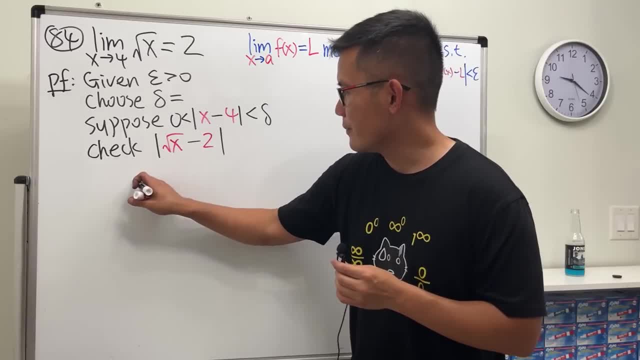 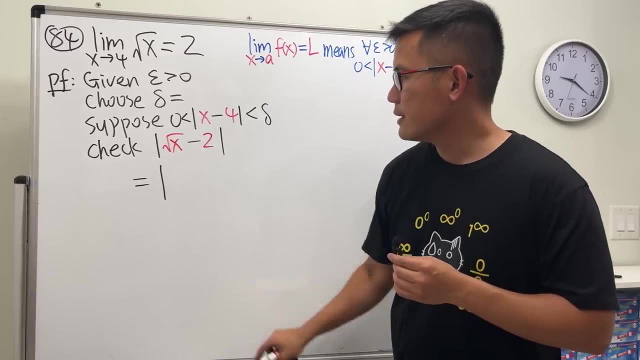 so let's go ahead and do that. i'm going to just write it down right here. i'm going to have square root of x minus. let me write it down like this: square root of x minus 2, right, and i'm going to multiply the top and 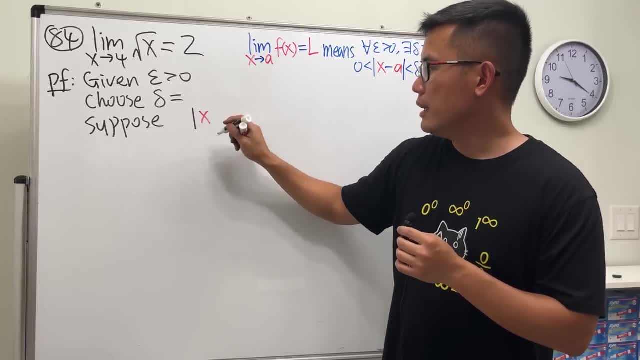 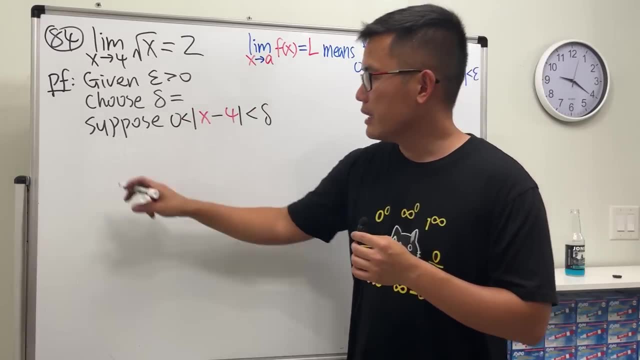 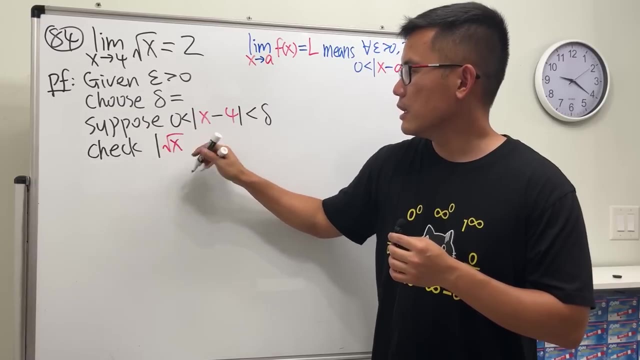 suppose what absolute value of x minus 4 to be less than delta and then greater than 0. Look backwards And then, lastly, we check absolute value function minus the limit. OK, that's all you have, All right now. 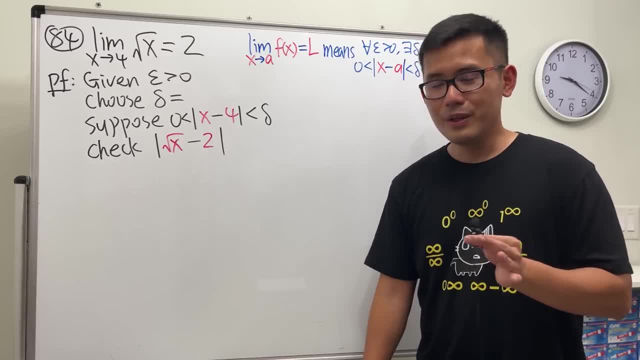 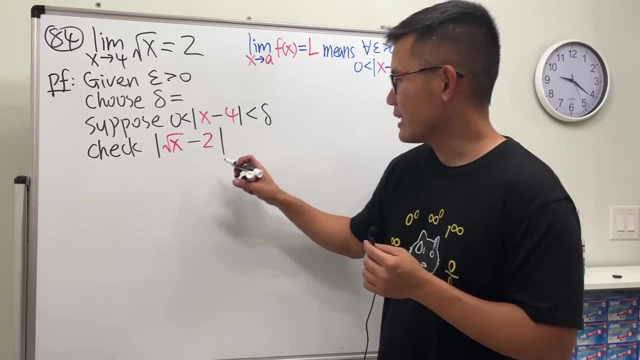 we cannot factor this anymore, But don't worry, We did a lot of this example before. When we have square roots, what did we do today? The count you get. So let's go ahead and do that. I'm going to just write it down right here. 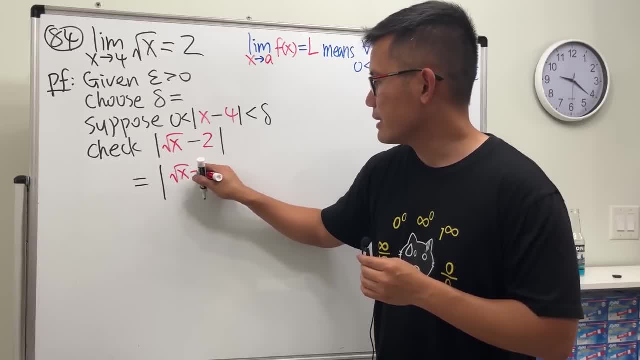 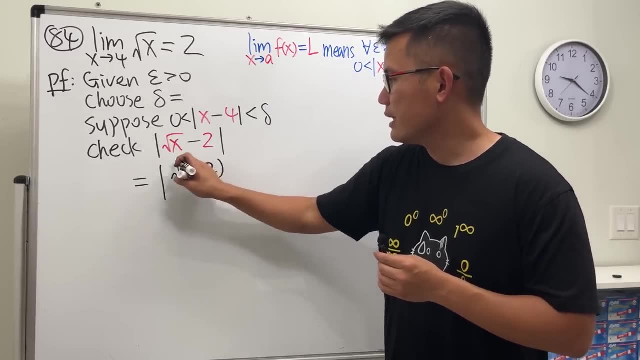 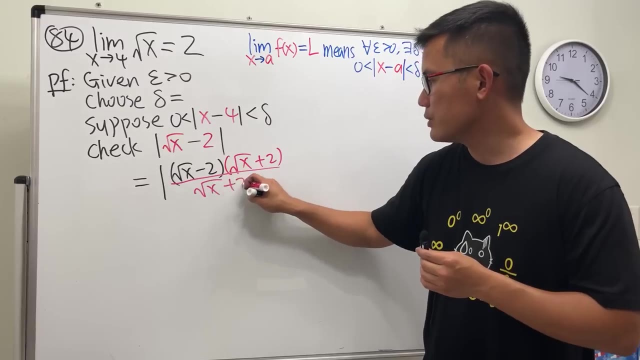 I'm going to have square root of x minus. Let me write it down like this: Square root of x minus 2, right, And I'm going to multiply the top and bottom by square root of x plus 2.. And then over square root of x plus 2.. 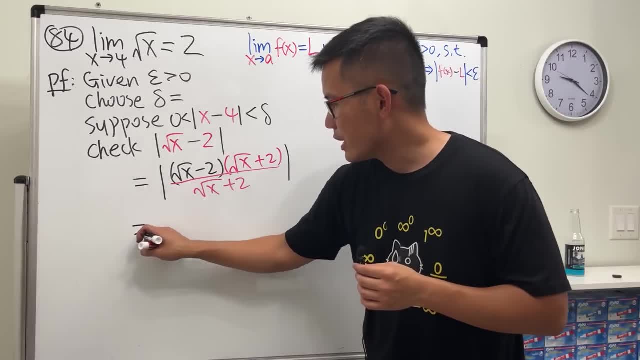 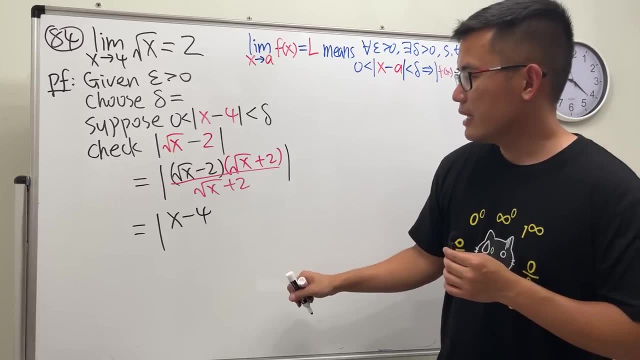 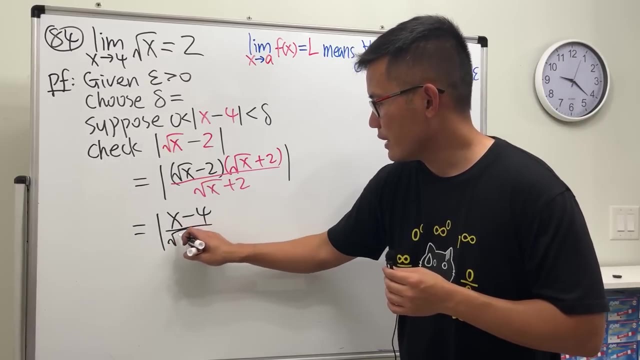 Aha, Yeah. And then you see this right here will give us just x on the top and then minus 4.. Right, So it's that. And then over square root of x plus 2. All right, So so far, so good. 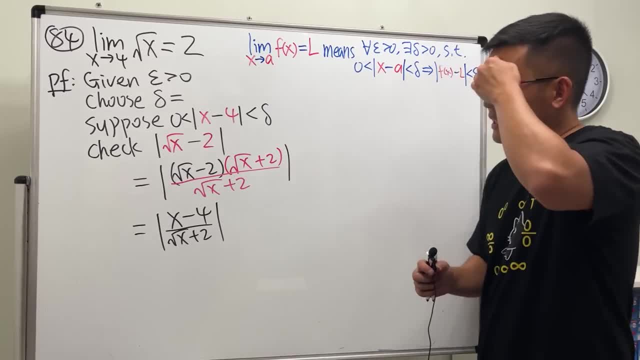 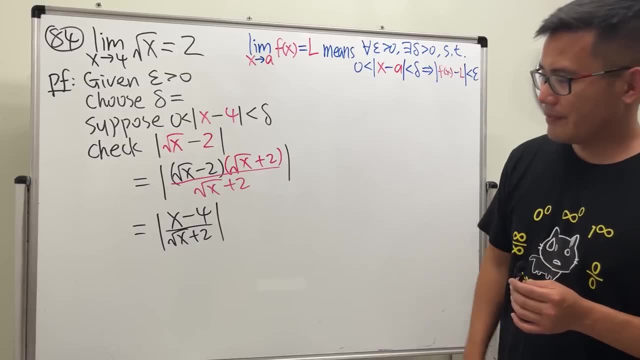 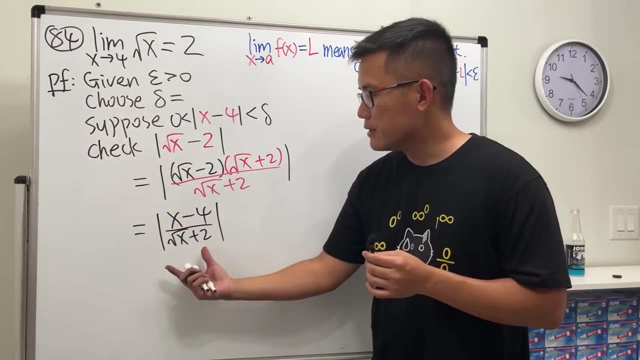 Take a look. Hopefully it's OK so far. It's hot, it's warm here, but it's OK, Almost done. What do we do next, though? Well, here's the thing: When we have an absolute value of a quotient, this, right here, is the same as 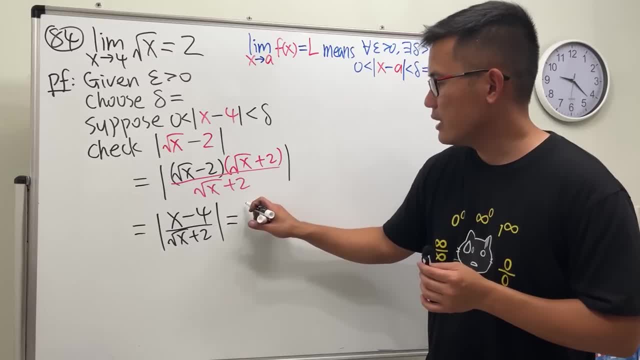 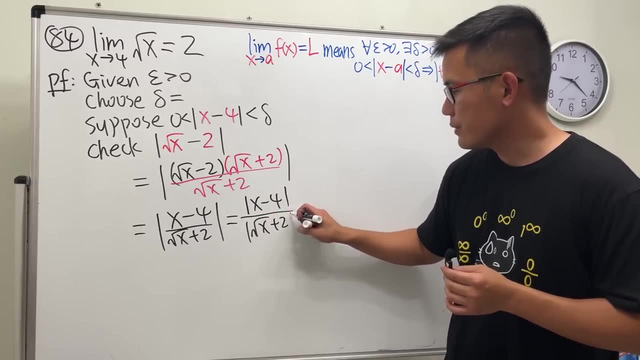 the quotient of the absolute value, meaning that we can look at this and say this is just the absolute value of x minus 4, and then over absolute value of square root of x plus 2.. But the thing is that the output of square root is always positive. 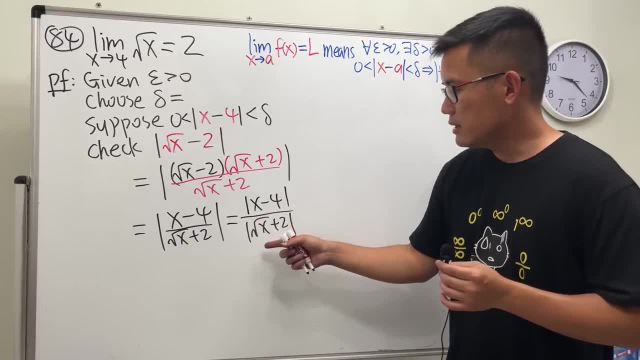 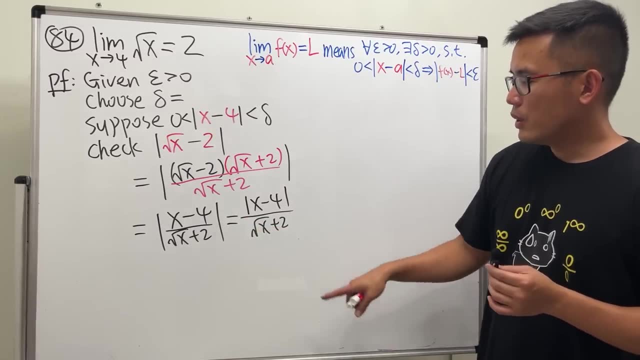 Likewise, when we add 2 to it, it's always positive. So this square root on the bottom doesn't matter. You can erase that. Good, And then you see, right here, this is the place that we can use the less than delta, which is yeah. 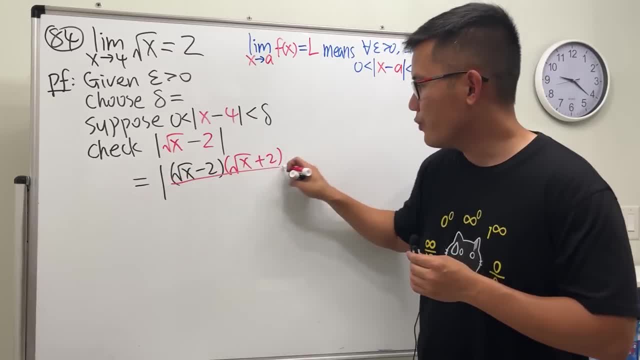 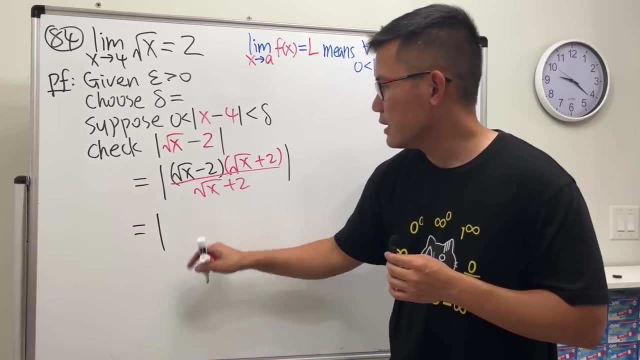 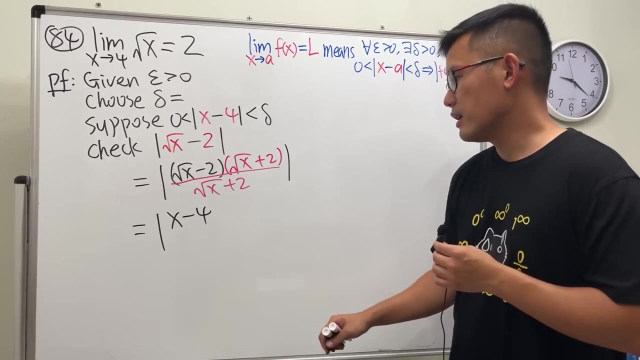 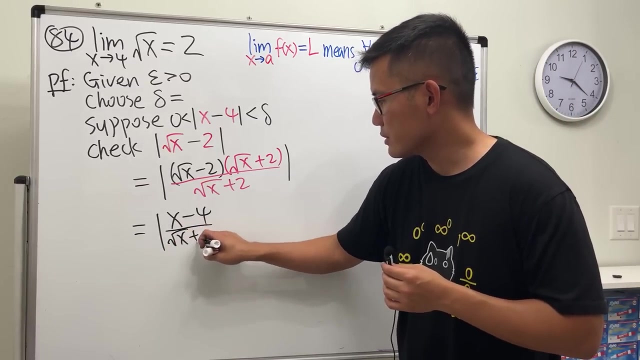 bottom, by square root of x plus 2, and then over square root of x plus 2.. aha, yeah, and then you see, this right here will give us just x on the top and then minus 4, right, so it's that, and then over square root of x plus 2.. all right, so so far, so good. 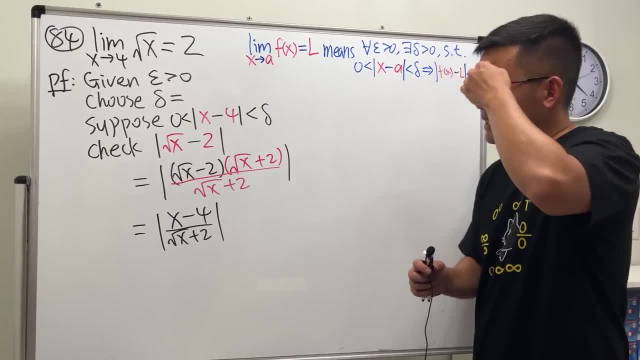 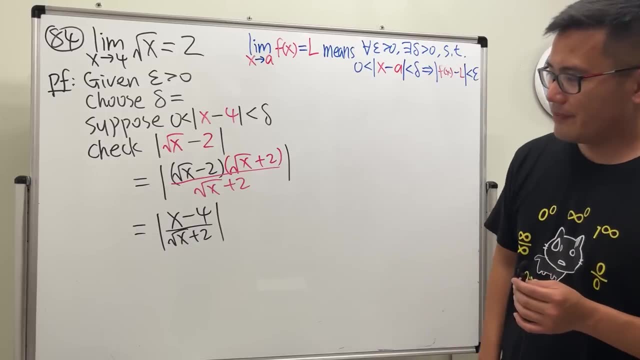 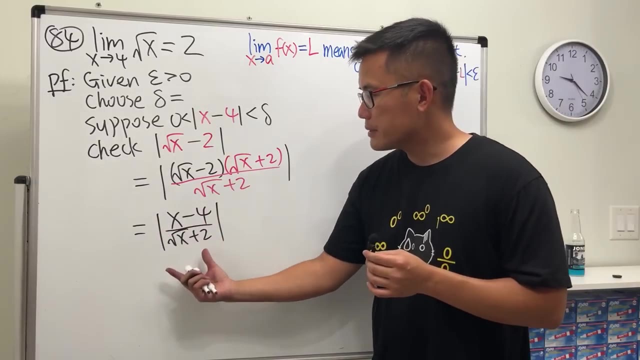 take a look. hopefully it's okay so far. it's hot, it's warm here, but it's okay, almost done. what do we do next, though? well, here's the thing: when we have an absolute value of a quotient, this, right here, is the same as the quotient of the absolute. 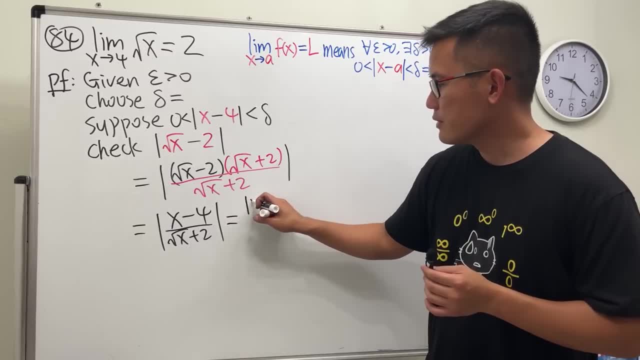 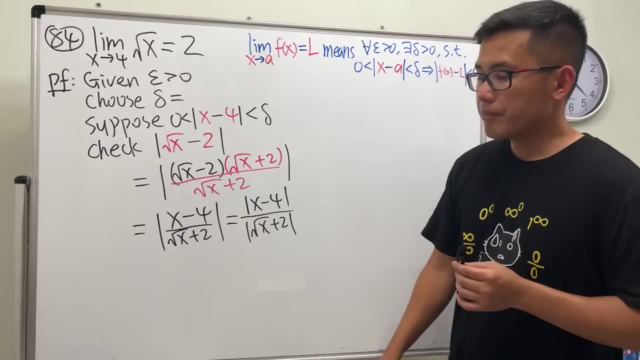 value, meaning that we can look at this and say: this is just the absolute value of x minus 4, and then over absolute value of square root of x plus 2.. but the thing is that the output of square root is always positive. likewise, when we add 2 to it, it's always positive. 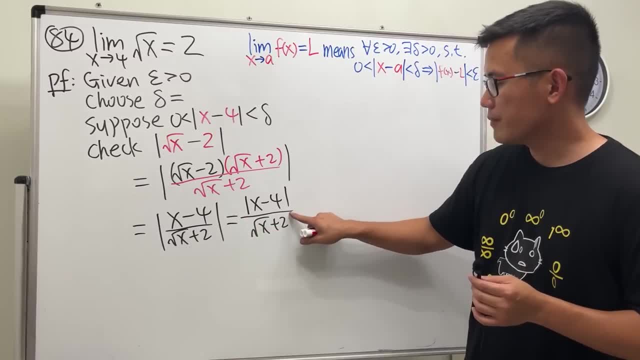 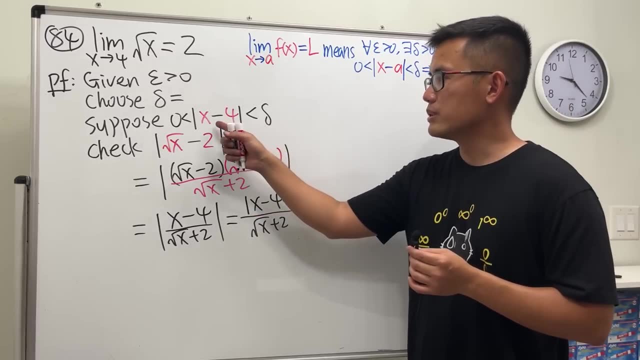 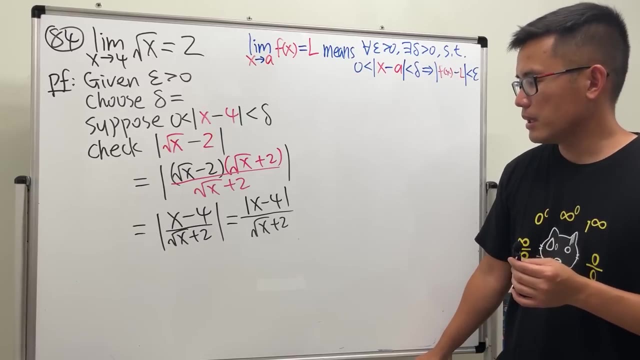 so this square root on the bottom doesn't matter, you can erase that. good. and then you see, right here, this is the place that we can use the less than delta, which is yay, but what exactly do we do with the button, though? we have square root of x plus 2.. 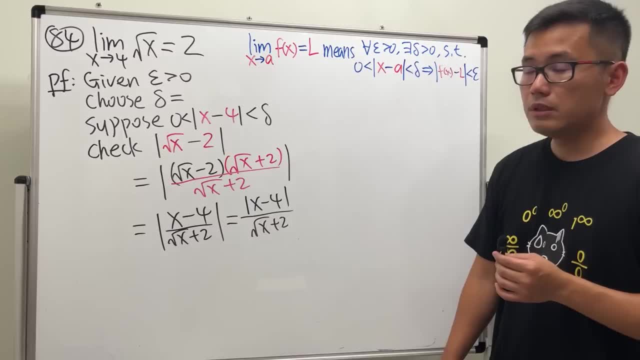 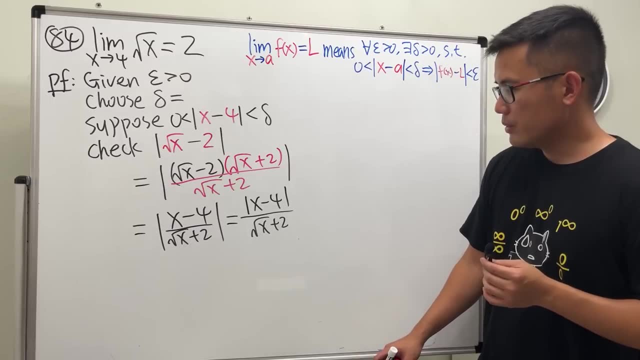 well, i'm actually just going to get rid of it. yeah, i'm just going to get rid of it, but you will have to say a few things for this, though, so i'm going to, um do like this. i think it's clear if i write it like this. 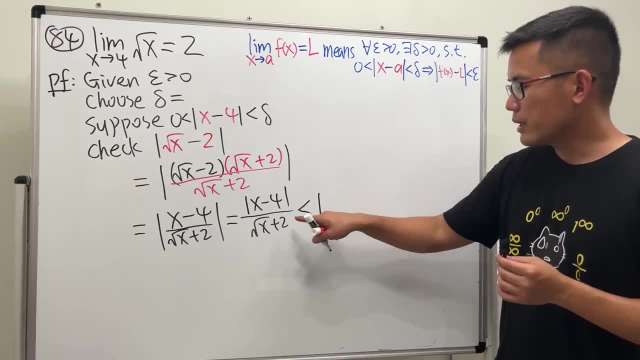 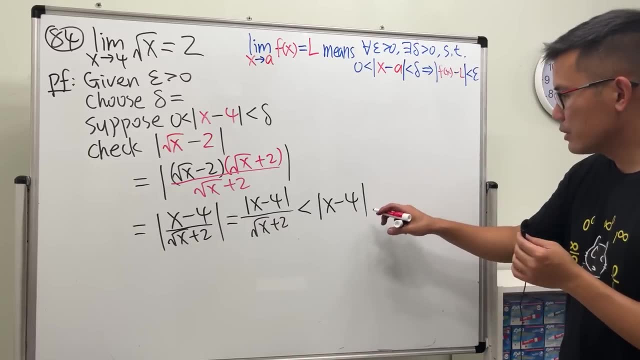 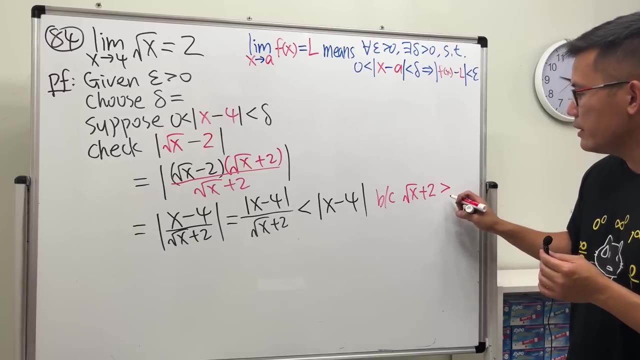 down right here. this right here is actually just equal to: so this right here is actually just less than absolute value of x minus 4.. just get rid of it why? i'm going to give you guys a explanation: because square root of x plus 2 is always greater than 1.. 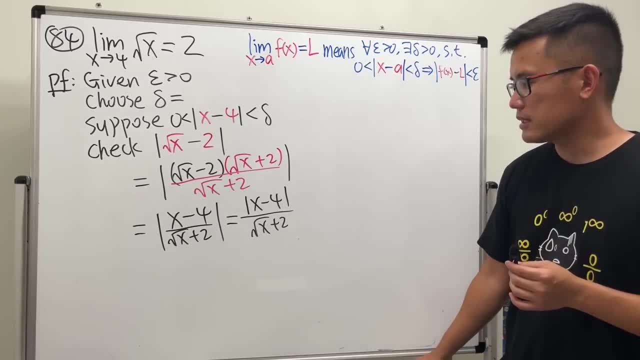 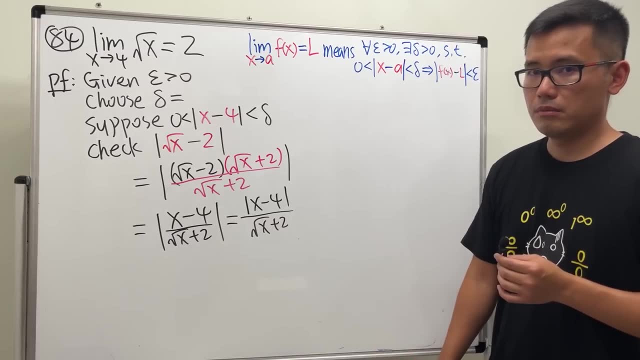 But what exactly do we do with the bottom? We have square root of x plus 2.. Well, I'm actually just going to get rid of it. Yeah, I'm just going to get rid of it, But you have to say a few things for this though. 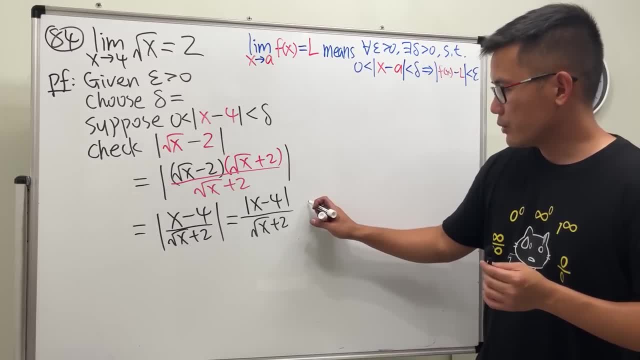 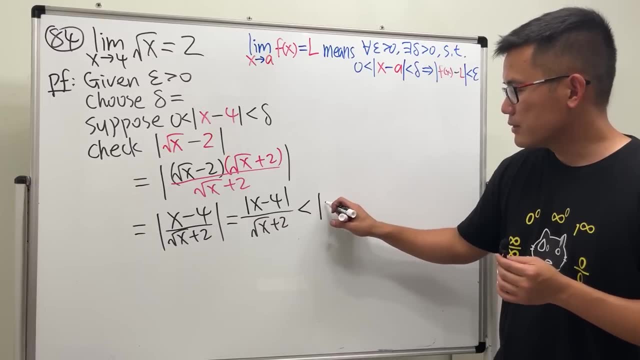 So I'm going to do like this. I think it's clear if I write it down here: This right here is actually just equal to: So this right here is actually just less than absolute value of x minus 4.. Just get rid of it. Why? 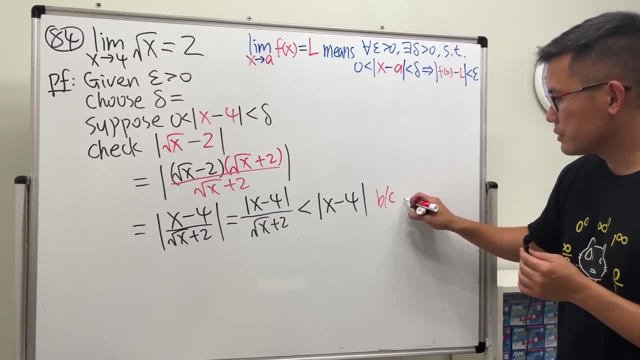 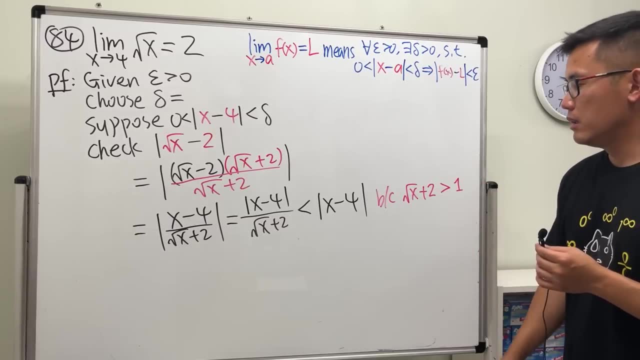 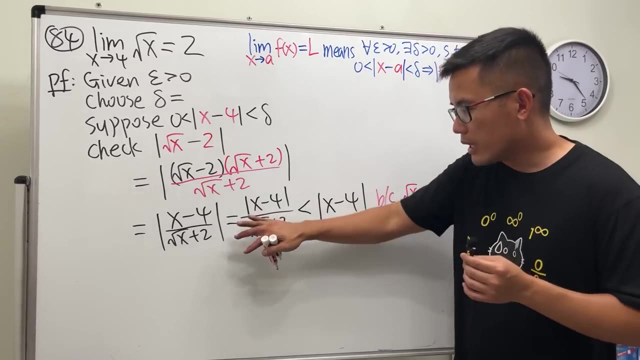 I'm going to give you guys an explanation, Because square root of x plus 2 is always greater than 1.. I'm not saying the bottom is always positive, I'm saying that the bottom is always greater than 1.. That's why, when I get rid of this, 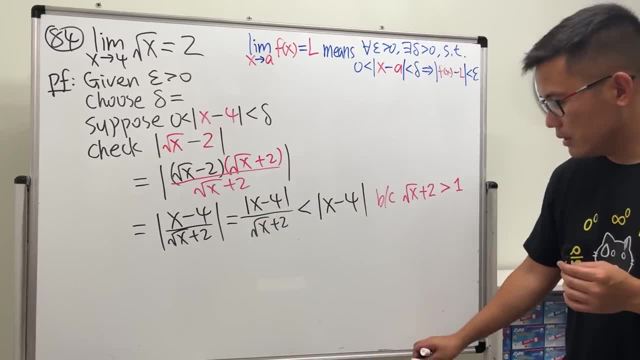 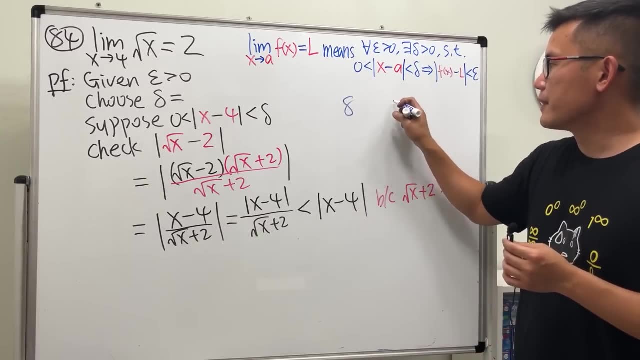 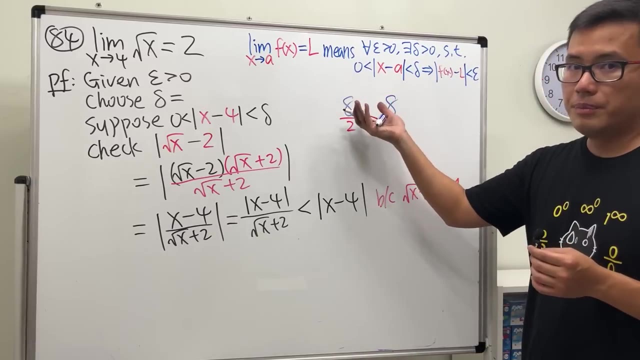 this right here is smaller than just the top. Let me give you an example to convince you guys. So suppose you have 8 versus 8.. Of course they are the same. But if today you have 8 and then divided by 2, then becomes what? 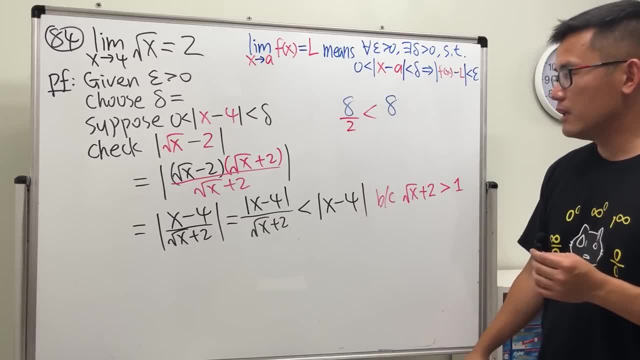 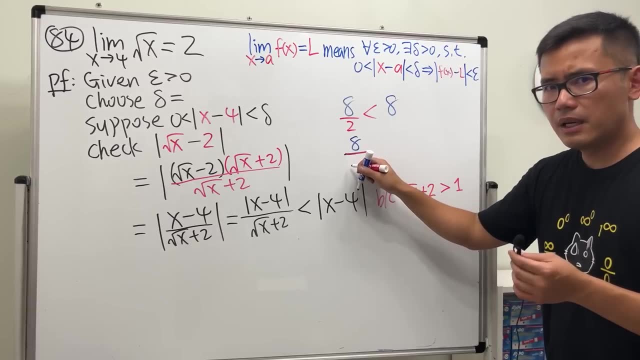 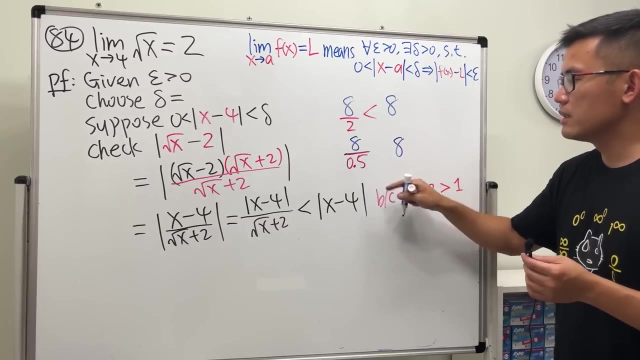 This right here becomes smaller than that, right Yeah. However, if you have 8 divided by, let's say, a number, that's positive, but it's 0.5 compared to 8, which one is bigger? This is bigger now. 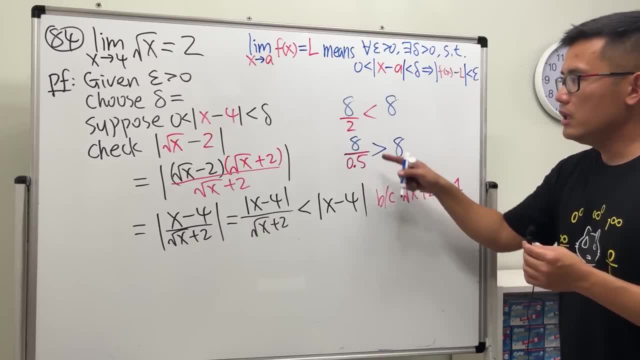 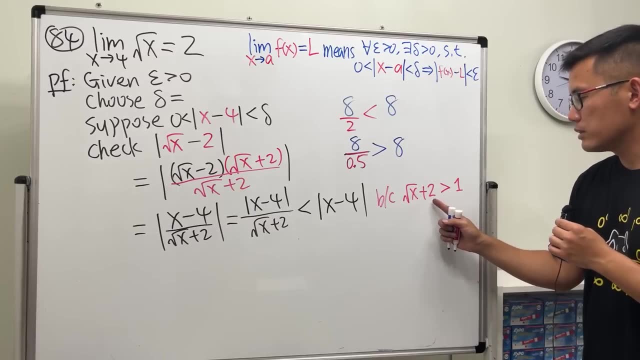 Yeah, If you divide it by 1, they are equal. If you divide it by a number that's bigger than 1, then this right here will be smaller than this. That's why I'm mentioning: square root of x plus 2 is bigger than 1.. 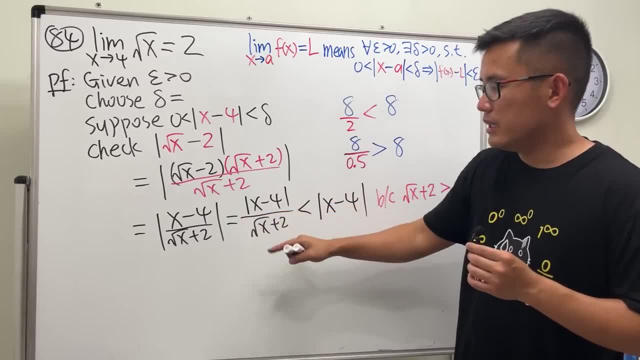 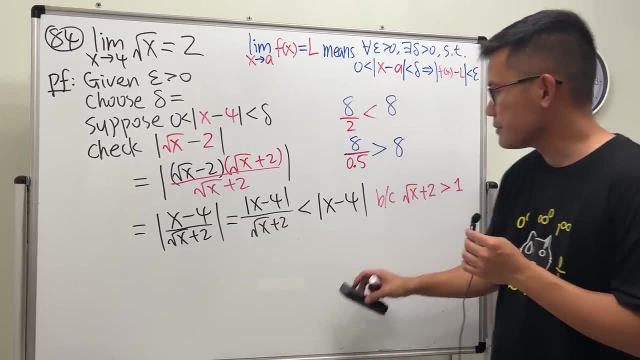 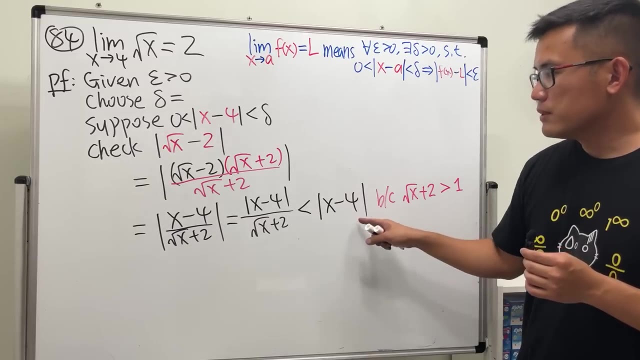 So I can legitimately get rid of the bottom and then just say: this is less than just the top, So this is the idea. So that should be clear, Right. So that's really really good, because now, when we have just the absolute value of x minus 4,. 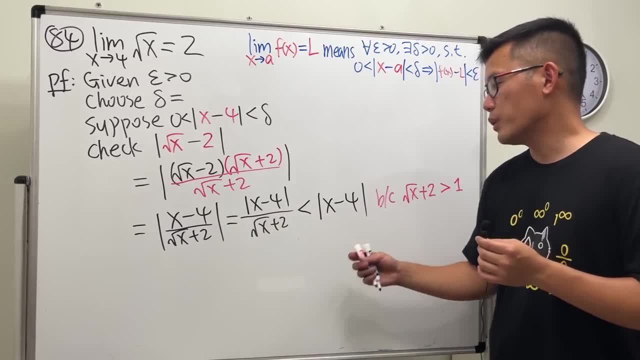 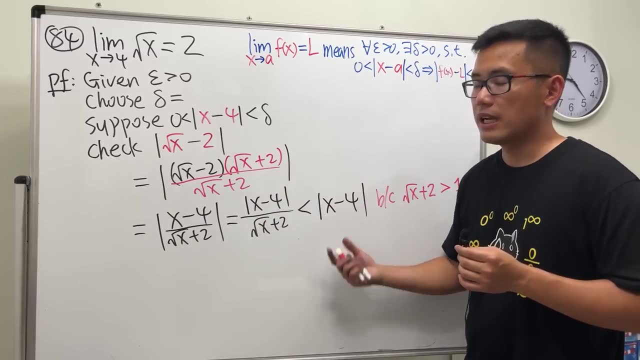 i'm not saying the bottom is always positive. i'm saying that the bottom is always greater than 1.. that's why, when i get rid of this right, this right here is smaller than just the top. let me give you an example to convince you, guys. 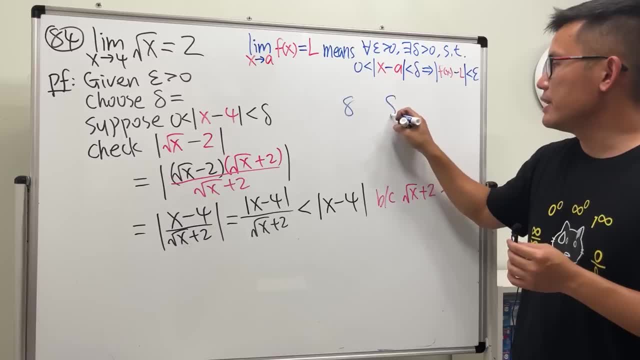 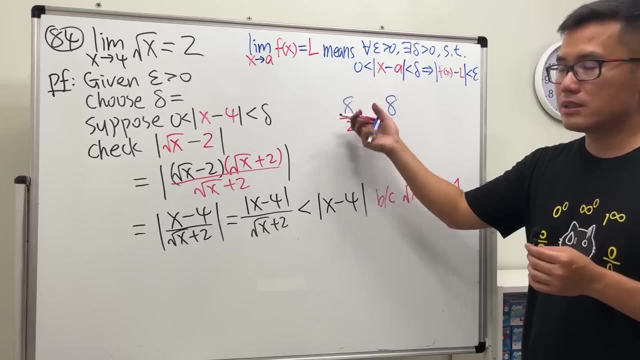 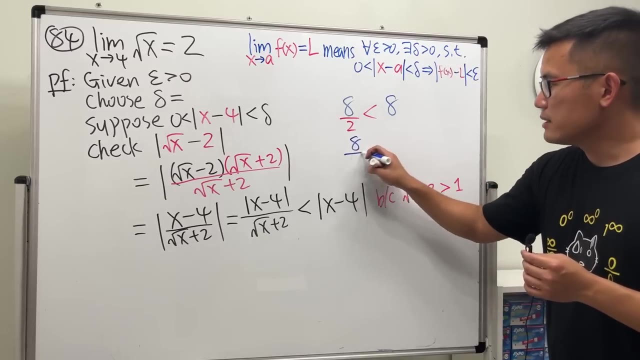 so suppose you have eight versus eight. of course they are the same. but if today you have eight and then divided by two, then becomes what? this right here becomes smaller than that, right, yeah. however, if you have eight divided by, let's say, a number, that's um. 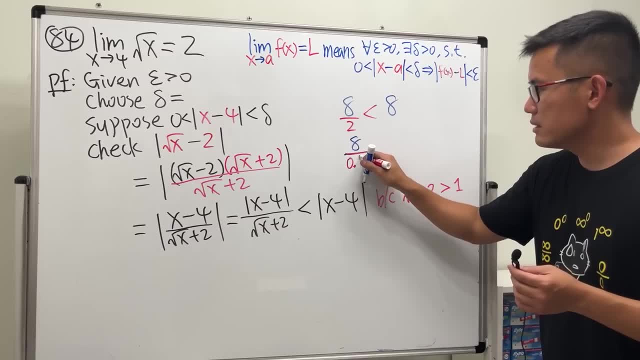 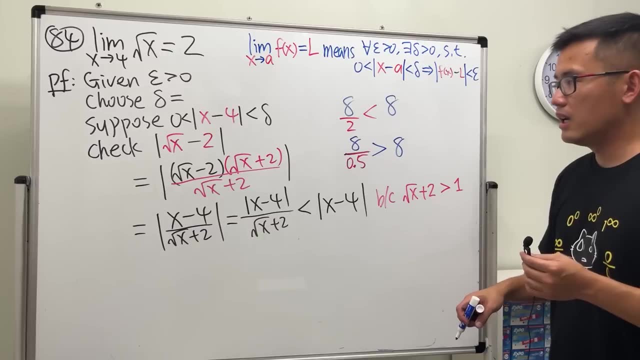 positive, but it's 0.5 compared to eight. which one's bigger? this is bigger. now. yeah, if you divide it by one, they are equal. if you divide it by a number that's bigger than one, then this right here will be smaller than this. that's why i'm mentioning square root of 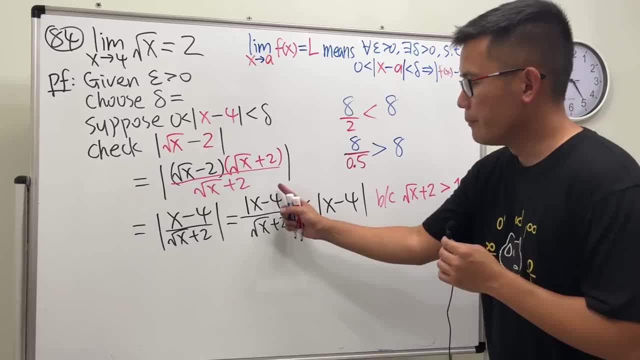 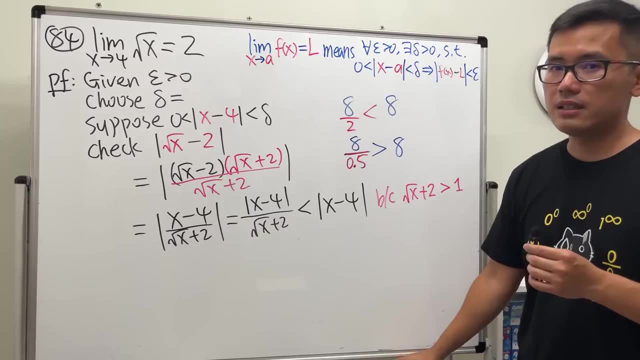 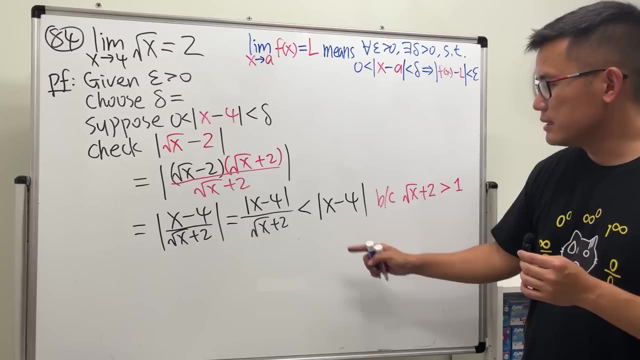 x plus 2 is bigger than 1.. so i can legitimately get rid of the bottom and just say this is less than just the top. so this is the idea. so that should be clear, right. so that's really really good, because now, when we have just the absolute four of x minus four, we can say this right: here is 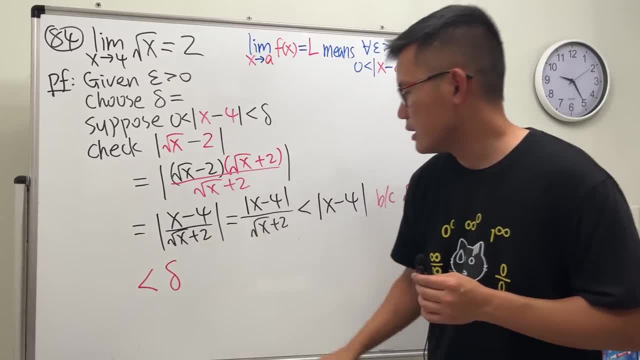 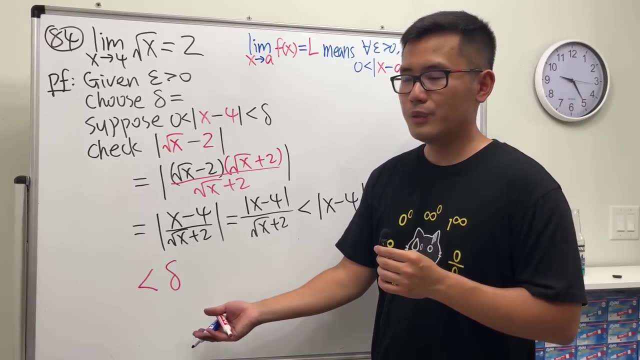 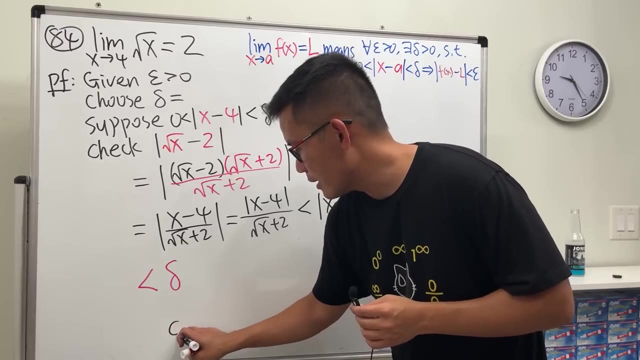 less than delta. now we can say: this is less than delta, yeah, and then what exactly do you want at the end? we just want this to be less than epsilon, right? so we want the whole thing right here to be like epsilon. so what do we want? we want delta to be equal. 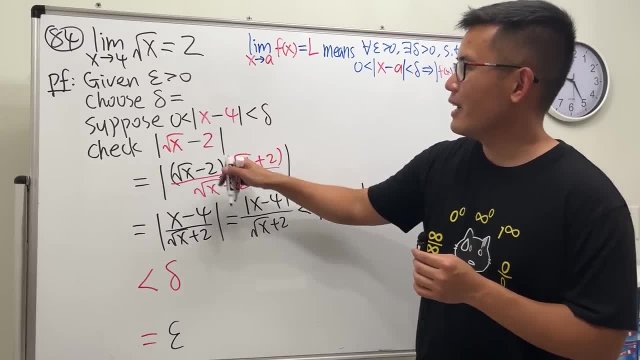 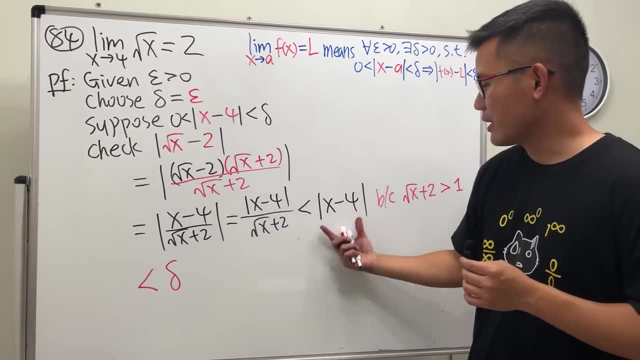 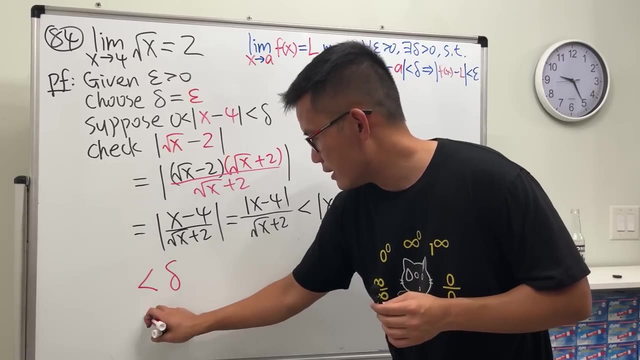 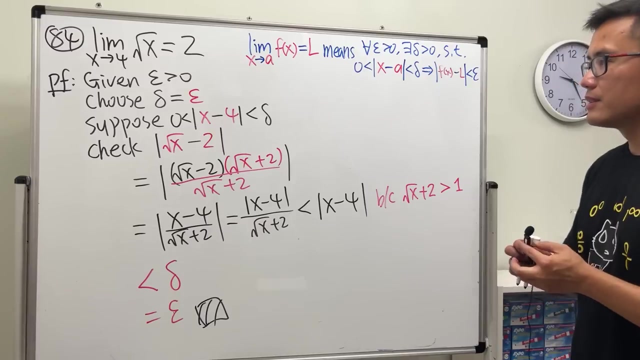 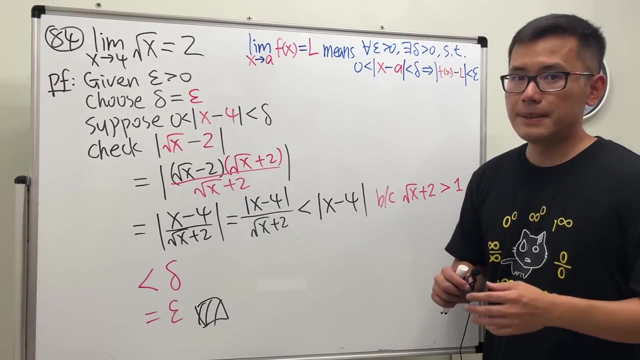 to epsilon. so we rush back here and just say delta is the same as epsilon and we are done. so this right here is less than delta, which is the same as epsilon, and we are done all right. so this right here might be a slightly difficult case, especially if you have not seen this kind of things before. but again, when we are 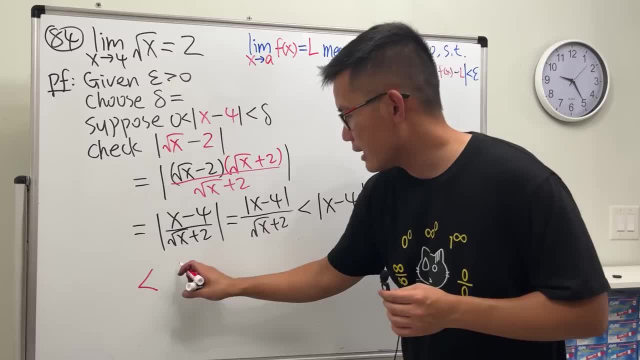 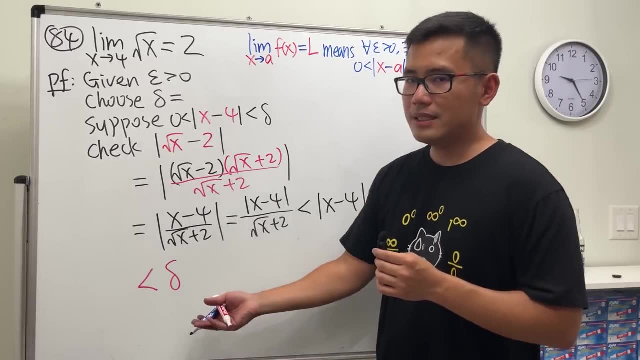 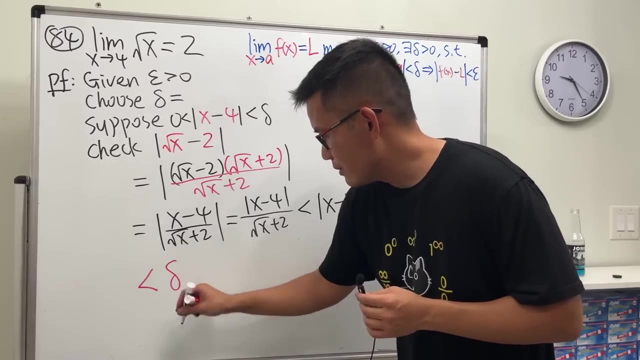 we can say: this right here is less than delta. Now we can say: this is less than delta, Yeah, And then what exactly do you want at the end? We just want this to be less than epsilon, right? So we want the whole thing right here to be like epsilon. 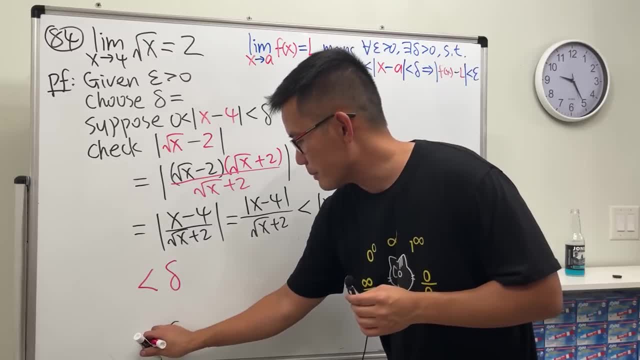 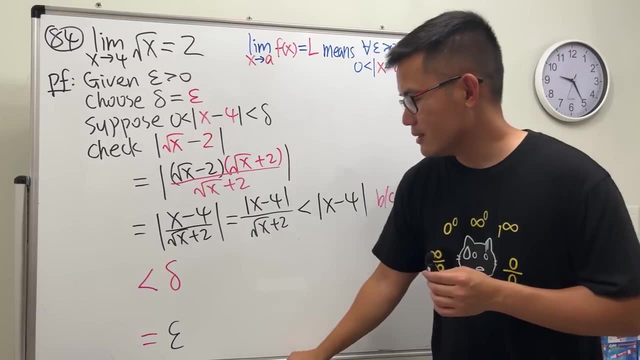 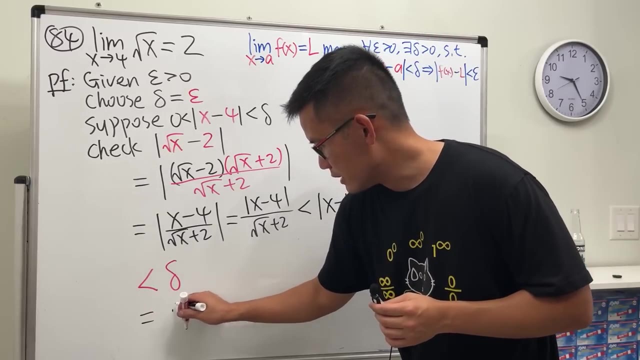 So what do we want? We want delta to be equal to epsilon. So we rush back here and just say delta is the same as epsilon, And we are done. So this right here is less than delta, which is the same as epsilon. 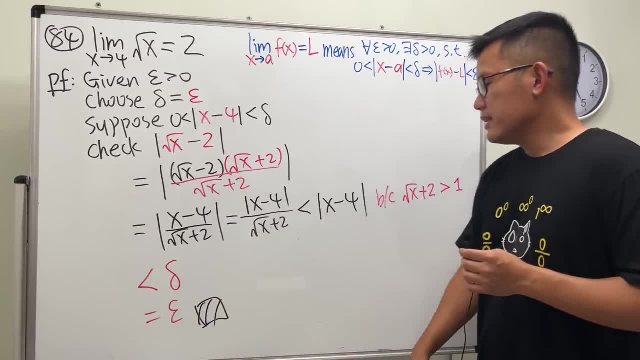 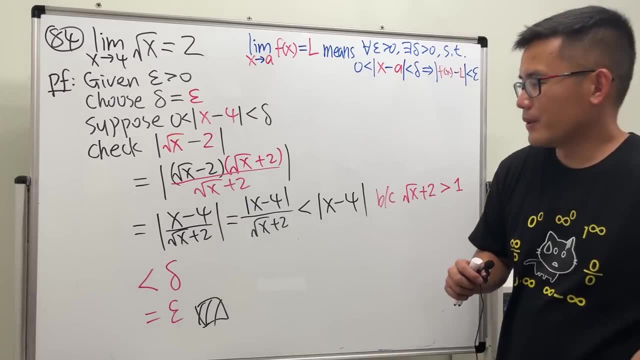 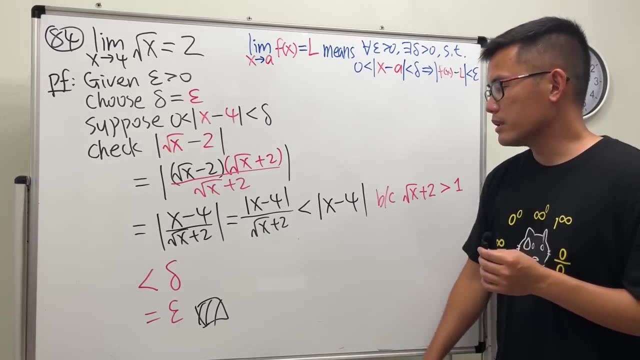 And then we are done All right. So this right here might be a slightly difficult case, especially if you have not seen this kind of things before. But again, when we are working with inequalities or absolute values, just be really careful. This is one of the things that we can do. 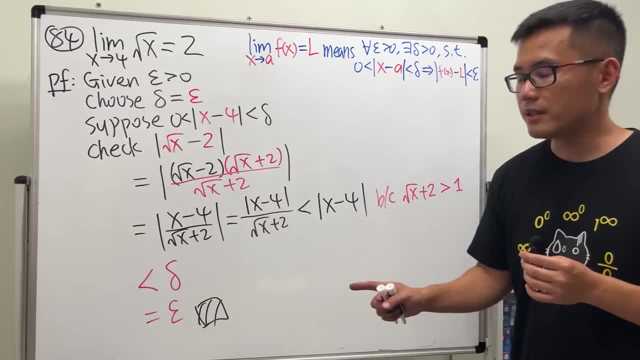 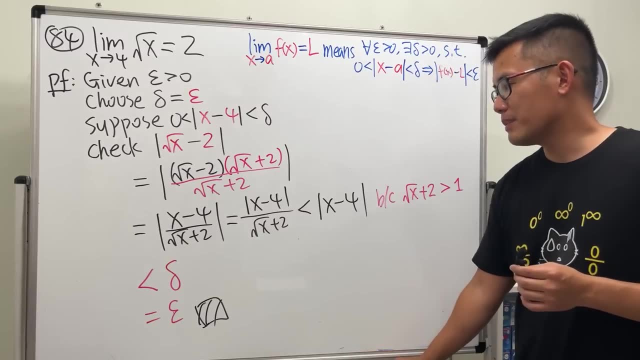 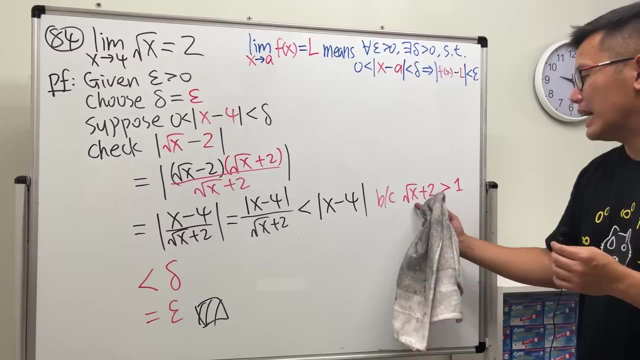 This is the key that simplifies this equation tremendously, Tremendously. If you don't use this, you can still do it other ways, like the ones that we are going to do later, But this is so much better Thanks to: square root of x is always positive, and then add 2 to it. 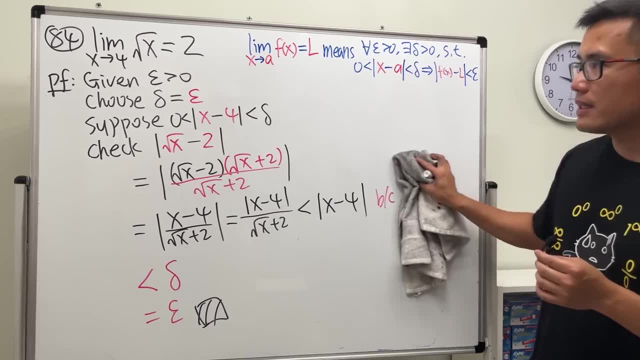 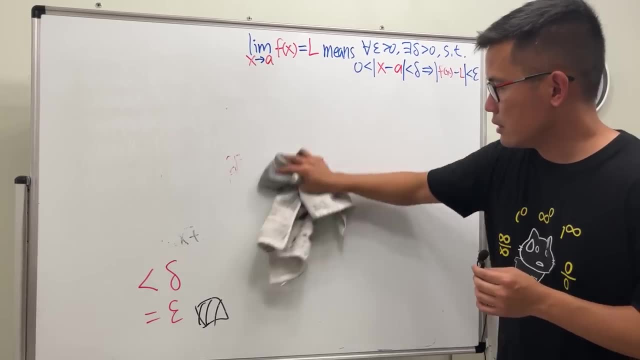 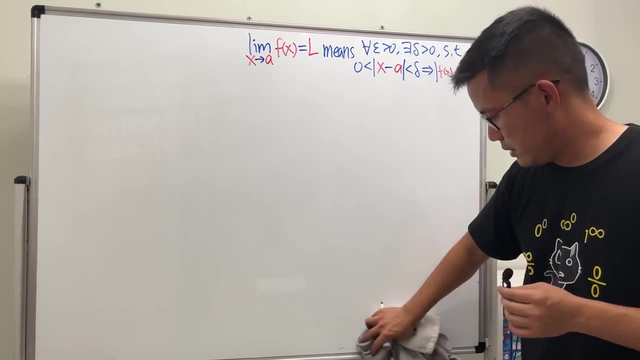 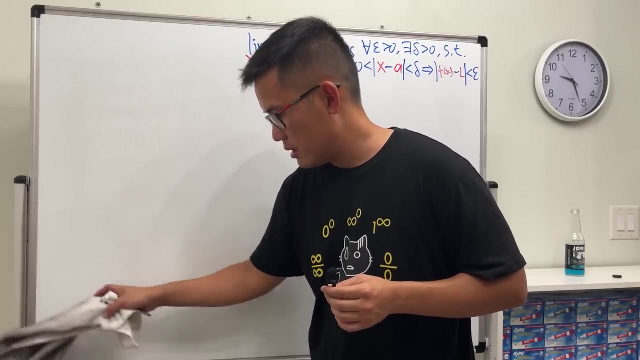 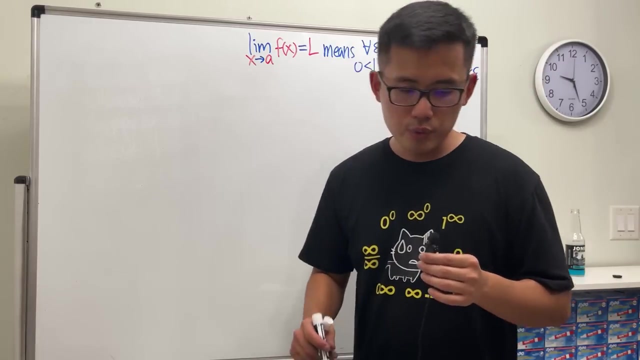 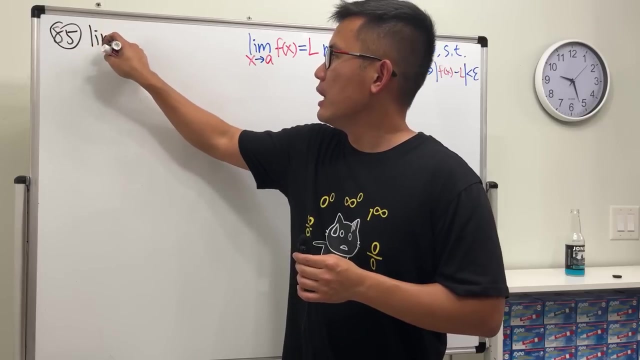 We know it's always greater than 1.. All right, So that's 84.. 옢- All right, 85,. another square root example, slightly trickier, slightly more complicated, but we can handle it. Limit as x approaching 6.. 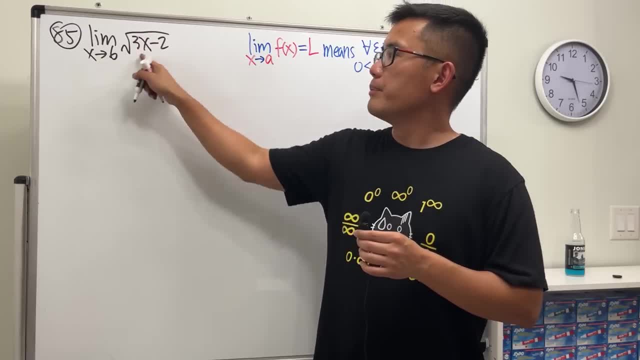 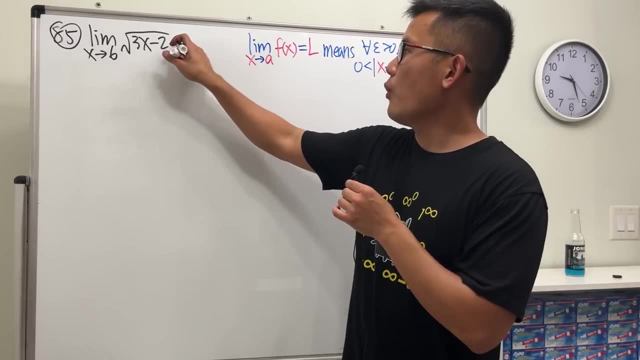 Square root of 3x minus 2.. Okay, put 6 in, here we get square root of 18 minus 2.. 18 minus 2 is 16.. Square root of that is 4.. Now prove it. 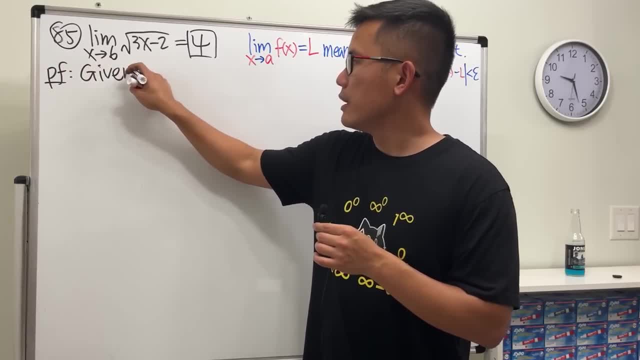 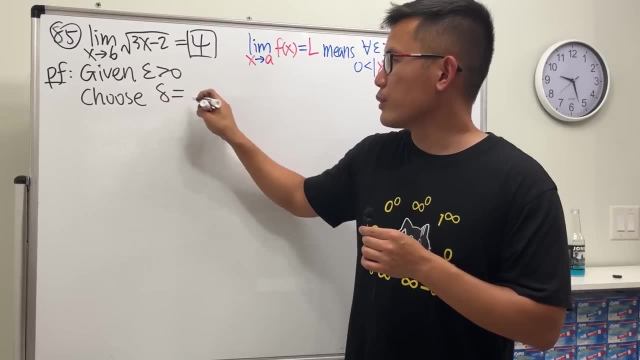 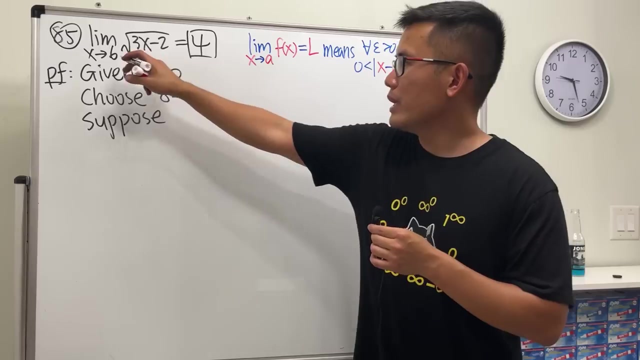 PF, given epsilon greater than 0.. Next we are going to choose delta. I don't know yet, so leave it. Then we are going to suppose Okay, and then we have x minus 6.. So just go ahead and put that in the absolute value. 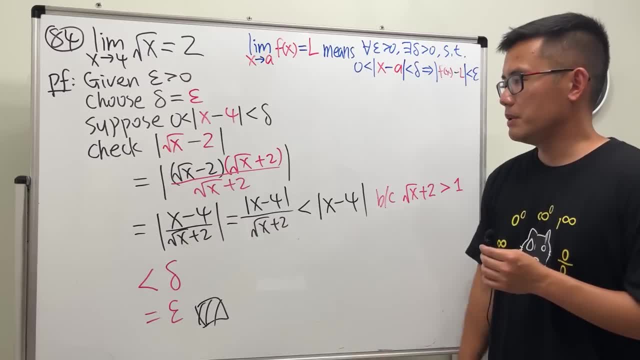 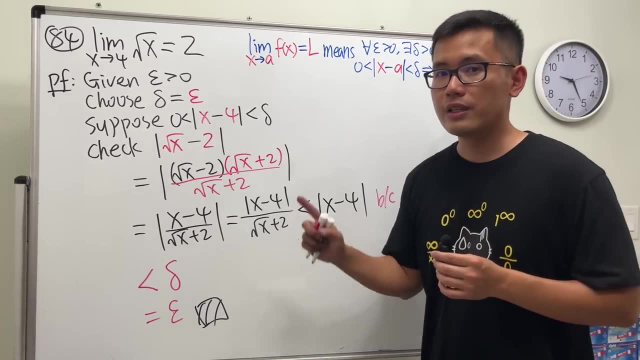 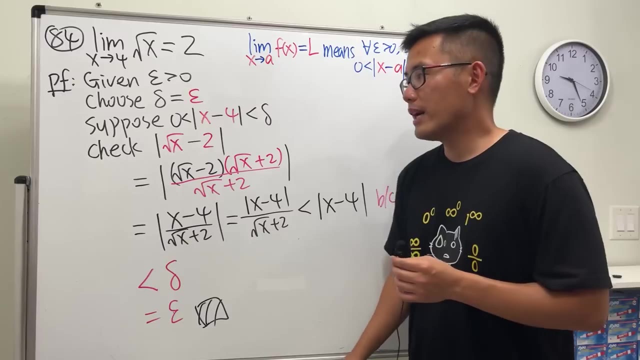 working with inequalities or absolute values. uh, just be really careful. this is one of the things that we can do. this is the key that simplifies this creation tremendously, draw tremendously. if you don't use this, you can still do it other ways, like the ones that we are going to do later, but 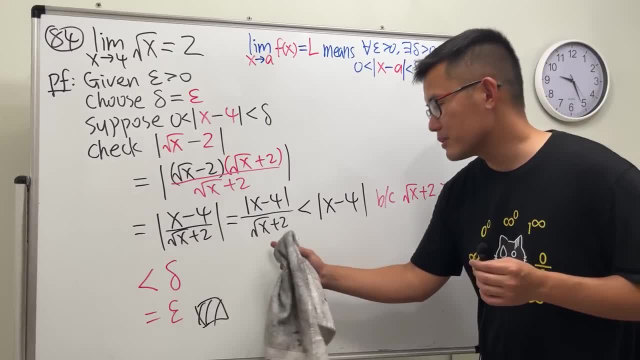 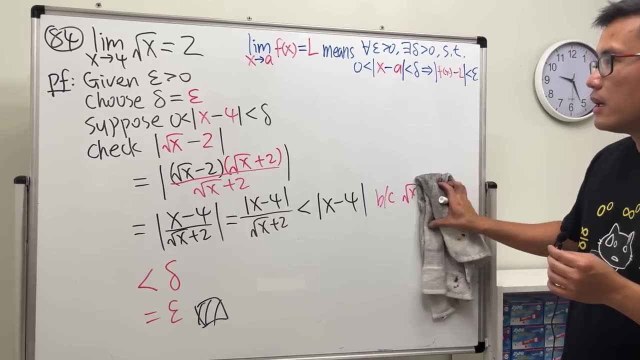 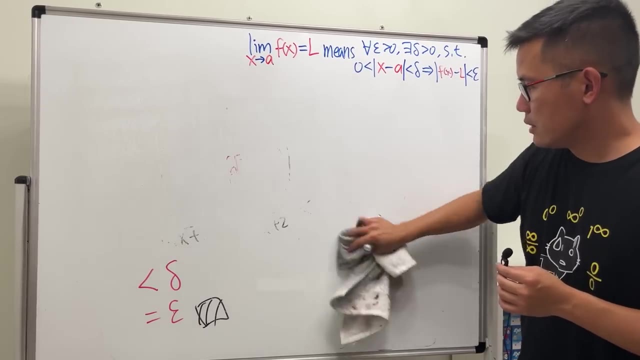 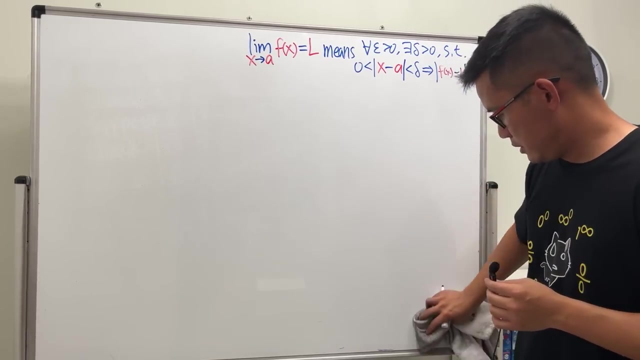 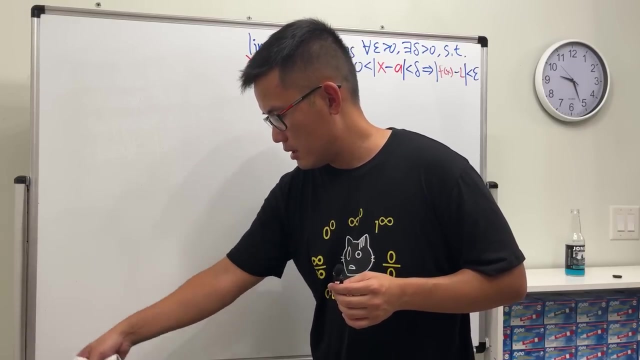 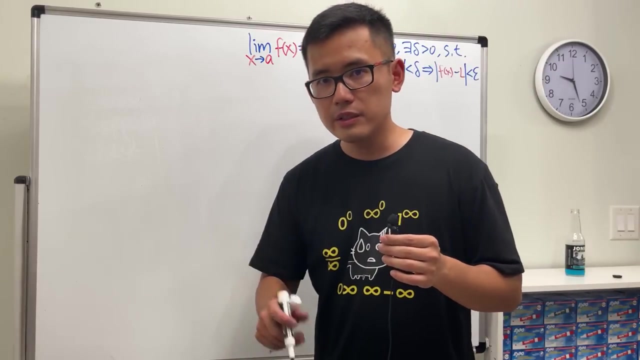 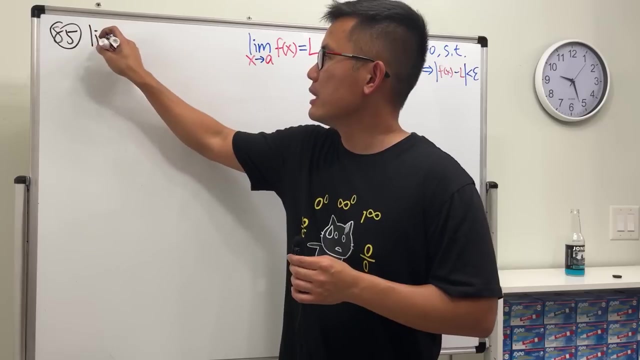 this is so much better thanks to absolute same, to: square root of x is always positive. and then add two to it, we know it's always greater than one. all right, so that's 84.. cm building, all right. 85. another square root example, slightly trickier. 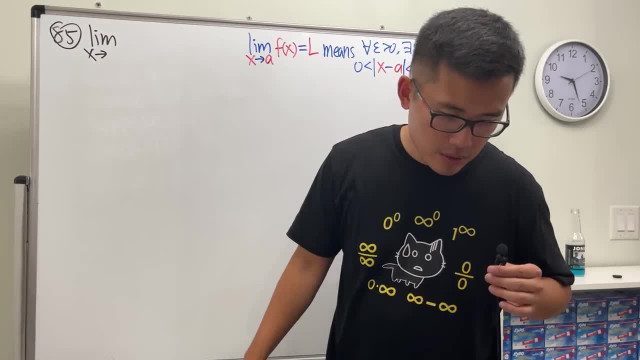 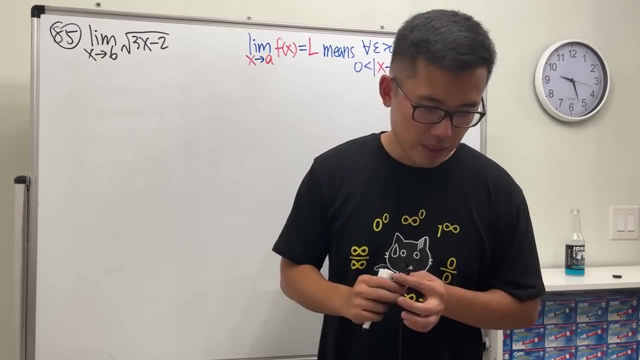 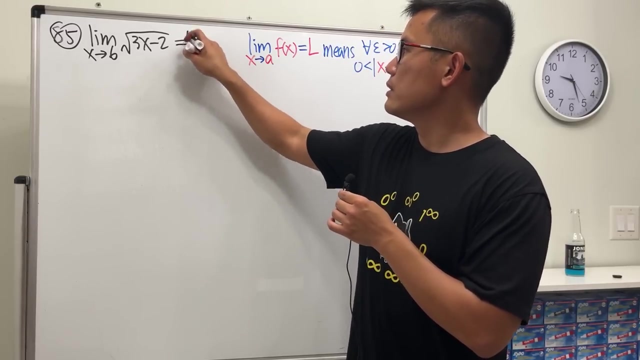 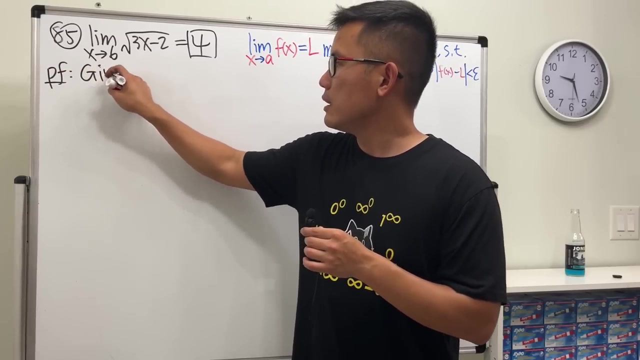 slightly more complicated, but we can handle it. limit as x approaching six. okay, put 6 in here we get square root of 18 minus 2. 18 minus 2 is 16. square root of that is 4. now prove it. p f given epsilon greater than 0. next we are going to choose. 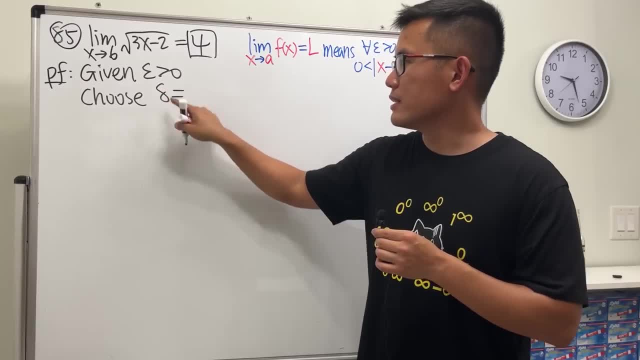 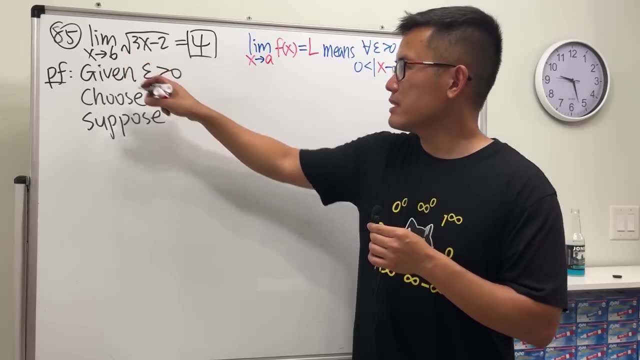 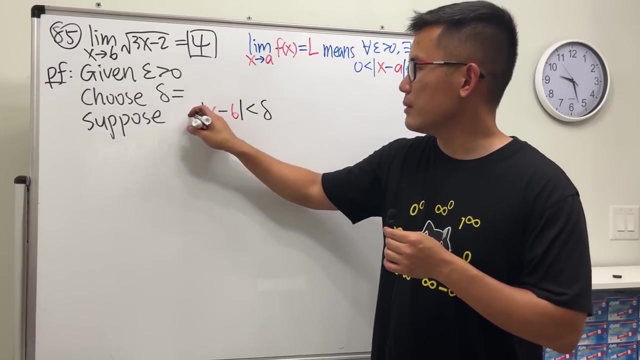 delta. i don't know yet, so leave it. then we are going to suppose okay, and then we have x minus 6, so just go ahead and put that in the absolute value and then this is less than delta and then greater than 0. then we are going to check. 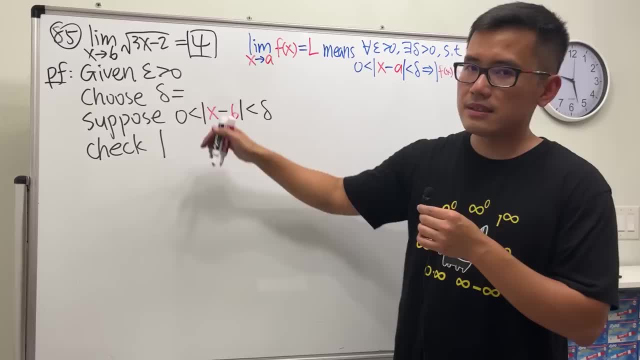 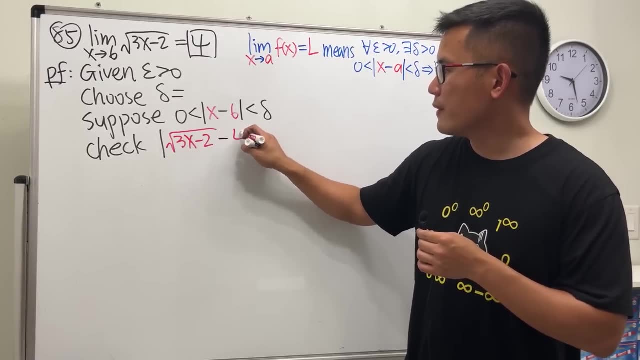 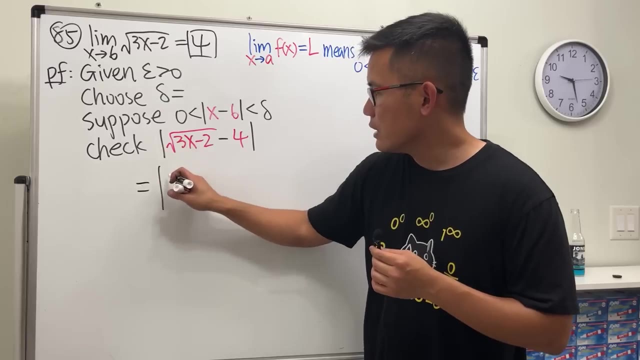 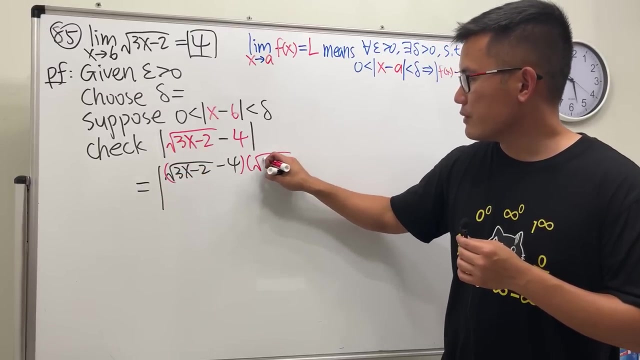 absolute value function minus the limit. so we have square root of 3x minus 2 minus 4. cool, now for this right here. do the conjugate business again. so this right here equals square root of root of 3x minus 2 minus 4. multiply the top and bottom by square root of 3x minus 2 plus 4. 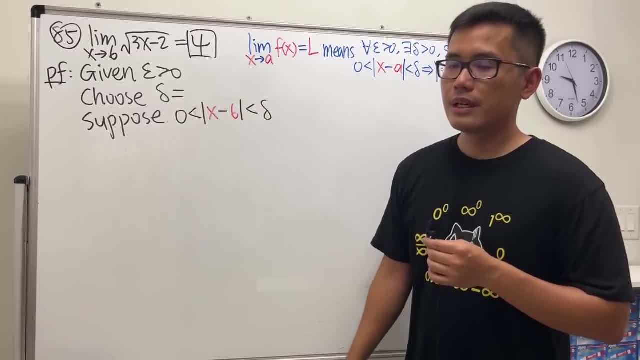 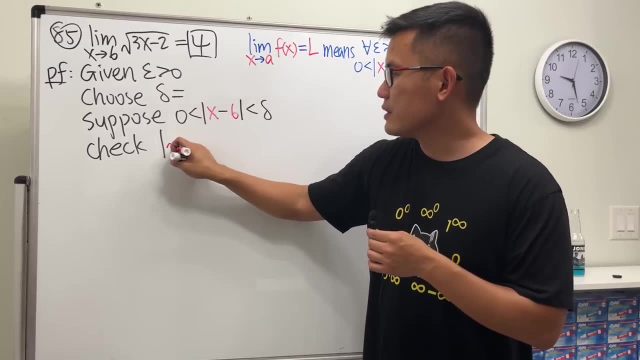 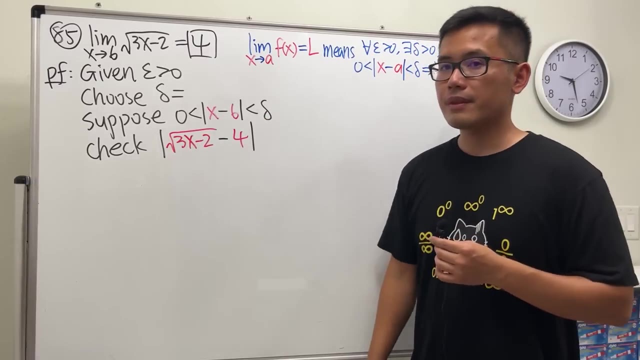 And then this is less than delta and then greater than 0. Then we are going to check absolute value function minus the limit. So we have square root of 3x minus 2 minus 4.. Cool, Now for this. right here, do the conjugate business again. 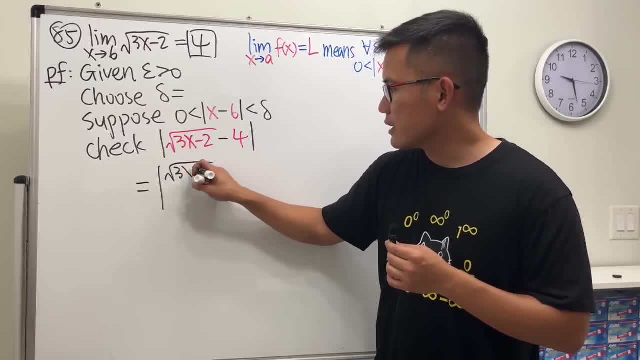 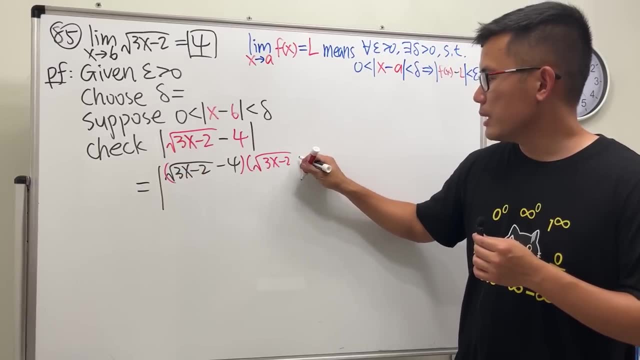 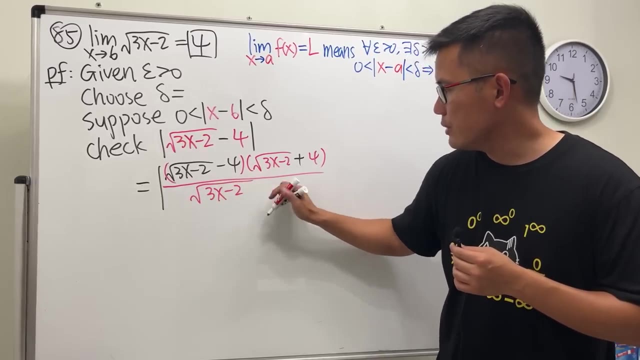 So this right here equals square root of 3x minus 2 minus 4.. Multiply the top and bottom by square root of 3x minus 2 plus 4.. And then do the same on the bottom as well: Square root of 3x minus 2 and then plus 4.. 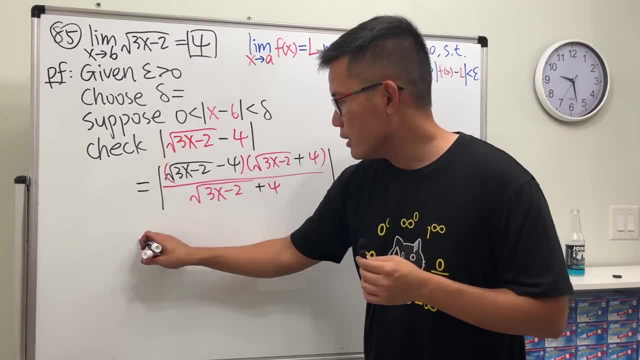 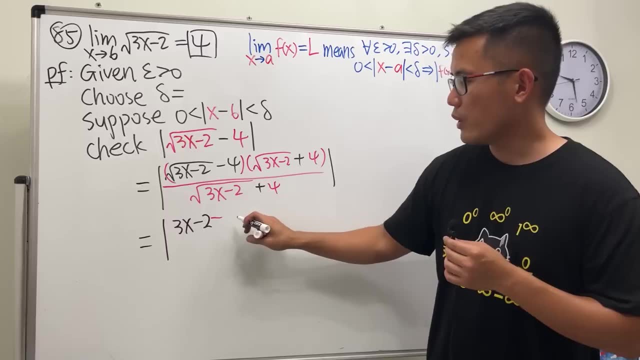 Cool. Now multiply out the top, We just get absolute value. It's just 3x minus 2 and then minus 4.. 4 squared, which is 16.. And then the bottom. we just keep it. So it's over square root. 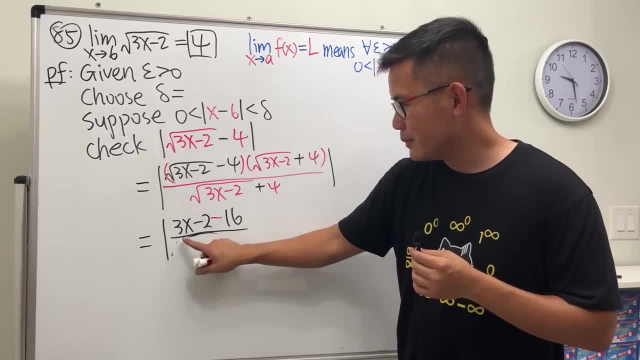 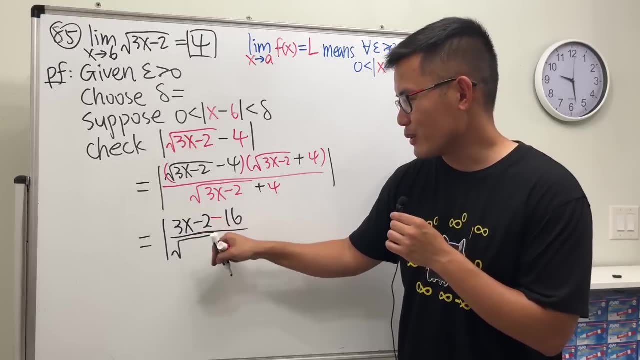 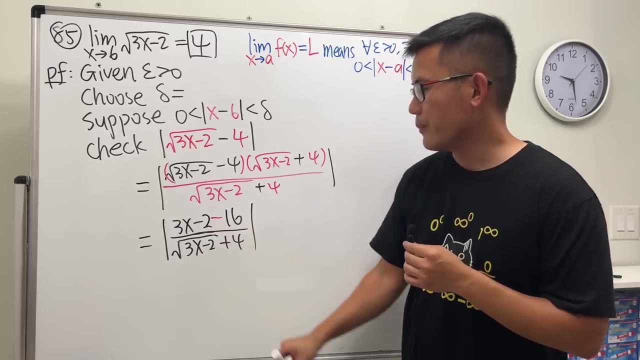 Ah, It's just over square root. There we go. I like to have a space between a square root and a sort of fraction bar 3x minus 2 and then plus 4.. Cool, Now let's do more algebra. 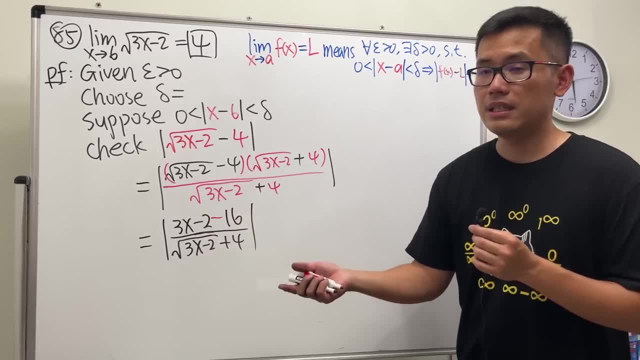 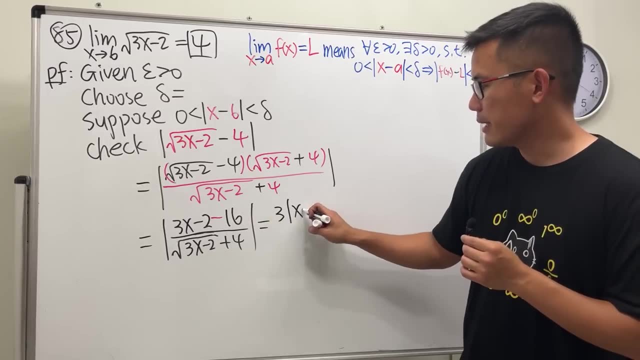 First of all we see that minus 2, minus 16. It's minus 18.. And then we can factor out 3. So on the top here we can have 3 absolute value, And then it's x minus 6.. 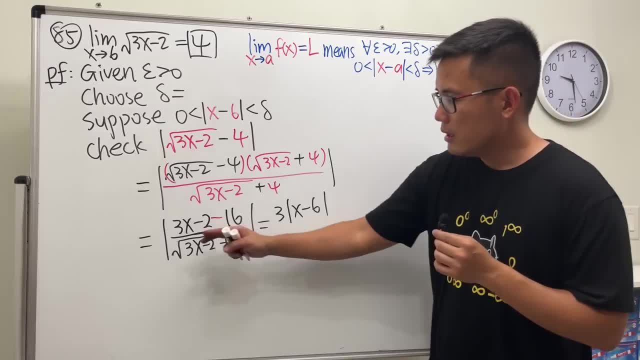 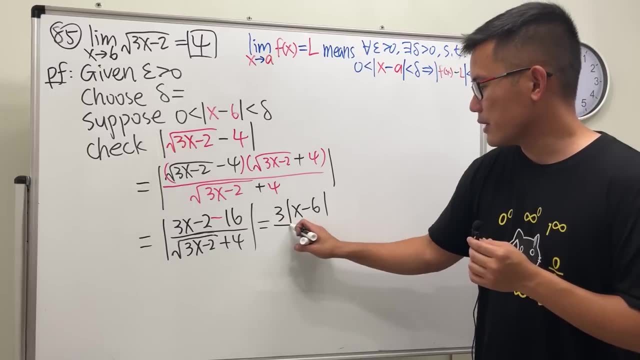 Okay, And then same idea like earlier: It's absolute value of the top and then absolute value of the bottom. But the bottom is always positive, So we don't need the absolute value, So we can just say square root of 3x minus 2 plus 4.. 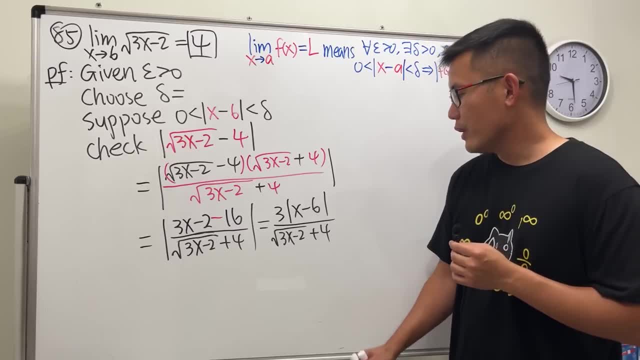 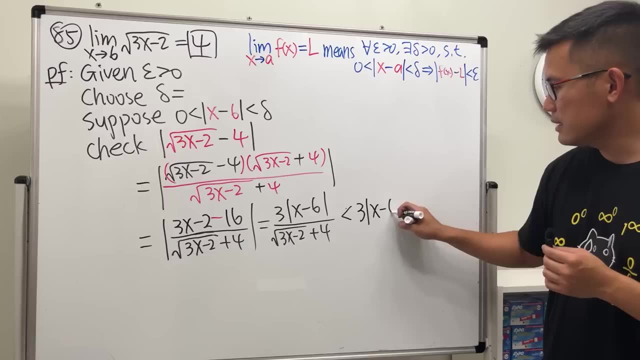 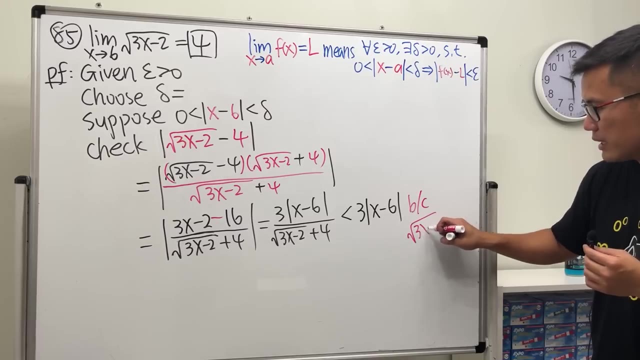 And what can we say next? Well, we can just get rid of the bottom part and say this: right, here is less than 3 times the absolute value of x minus 6.. Why? Because we will mention that square root of 3x minus 2 plus 4 is greater than 1.. 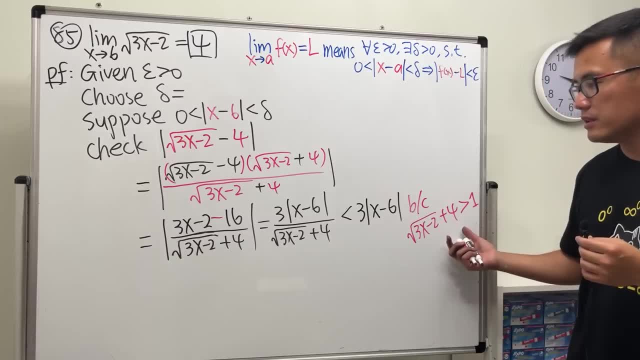 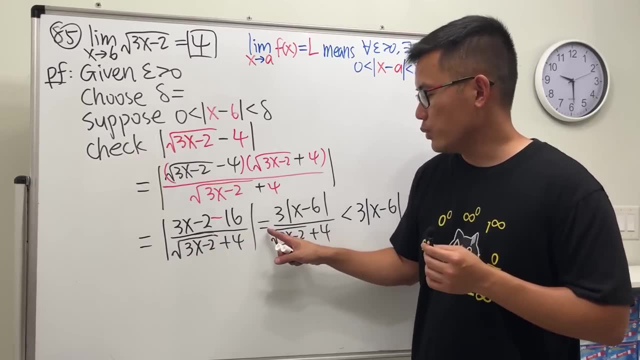 Right. That's why you have to mention. You don't mention this is greater than 0.. You mention: this is greater than 1.. From here to here, we mention it's greater than 0 because we can get rid of the absolute value. 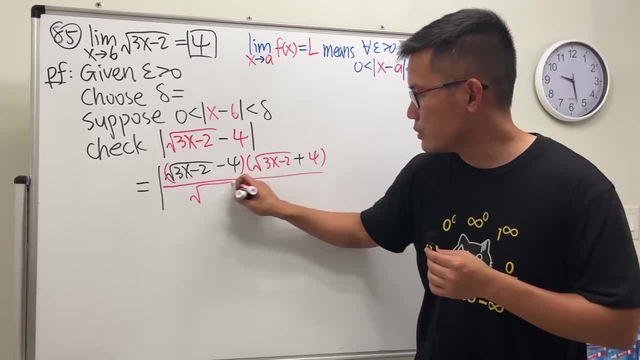 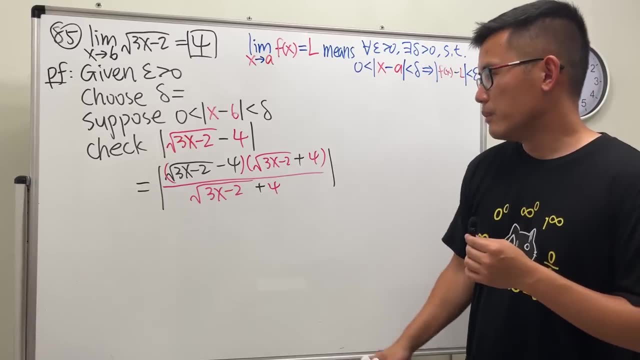 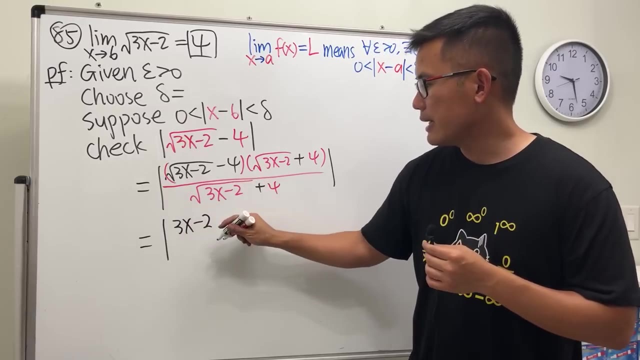 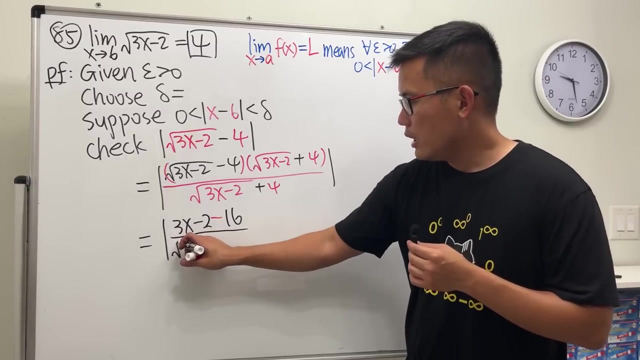 and then do the same on the bottom as well. square root of 3x minus 2 and then plus 4. cool, now multiply out the top, we just get absolute value. it's just 3x minus 2 and then minus 4, square, which is 16. and then the bottom. we just keep it, so it's over square root. 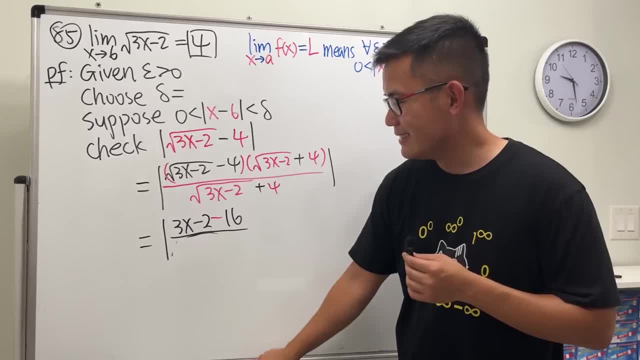 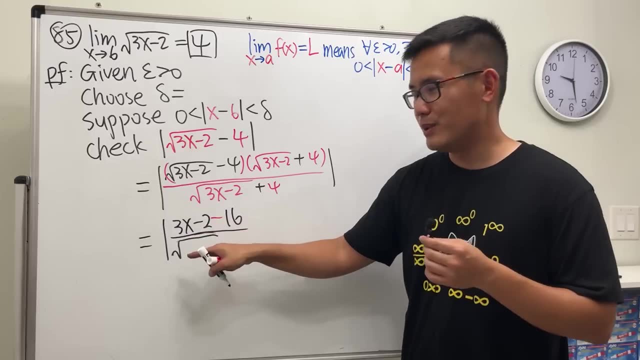 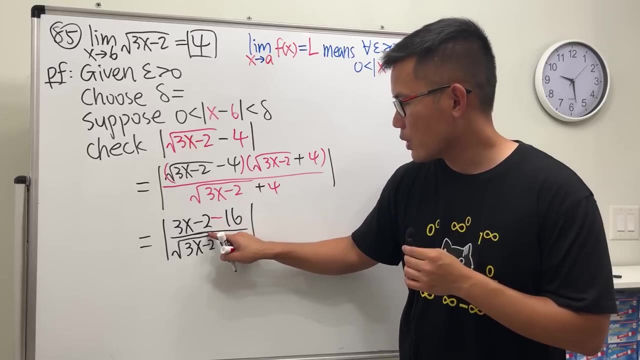 it's just over square root. there we go. i like to have a space between a square root and a solar fraction bar 3x minus 2, and then plus 4. cool, now let's do more algebra. first, though, we see that minus 2, minus. 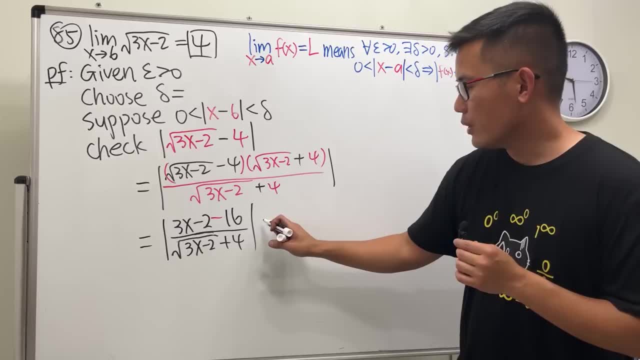 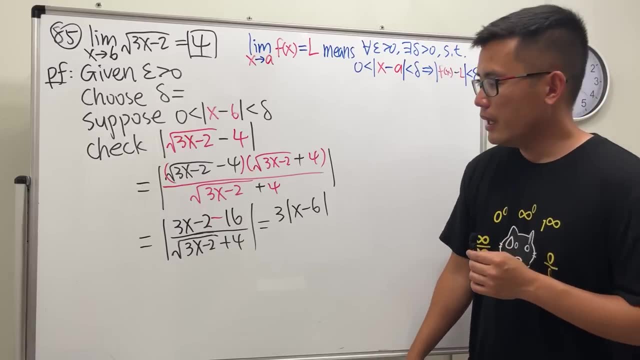 6, 16 is minus 18, and then we can factor out 3, so on the top here we can have 3 absolute value, and then it's x minus 6, okay, and then same idea like earlier, it's an absolute value of the top. 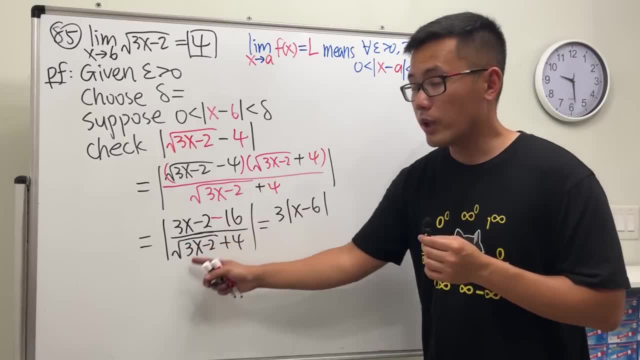 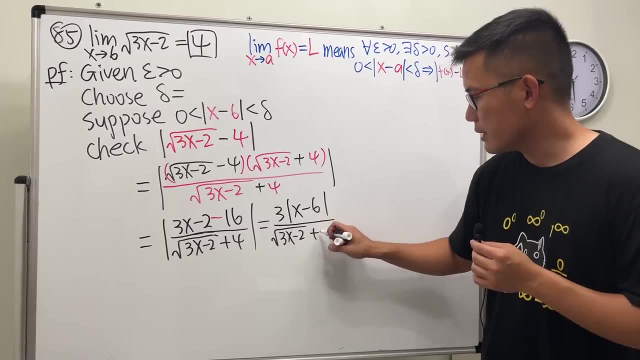 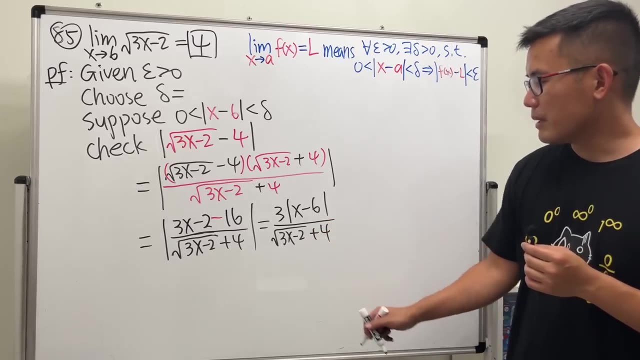 and then absolute value of the bottom. but the bottom is always positive, so we don't need the absolute value. so we can just say: square root of 3x minus 2 plus 4. and what can we do? what can we say next? well, we can just get rid of the bottom part and say this right here is less than 3 times the absolute. 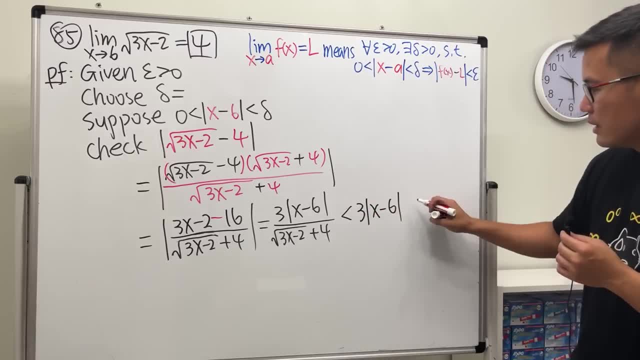 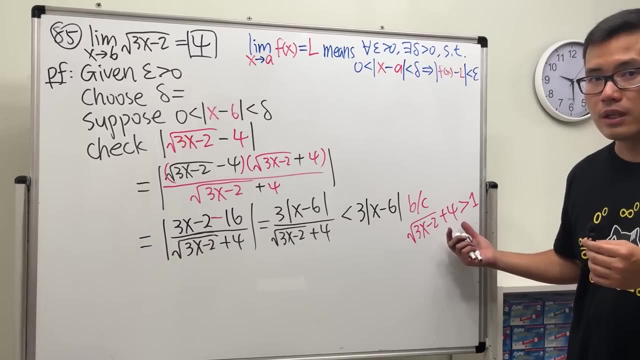 value of x minus 6. why? because- and we will mention that square root of 3x minus 2 plus 4 is greater than 1, right? that's why you have to mention, you don't mention this is greater than 0. you mention this is greater than 1. from here to here, we mention it's greater than 0 because we can get rid of the. 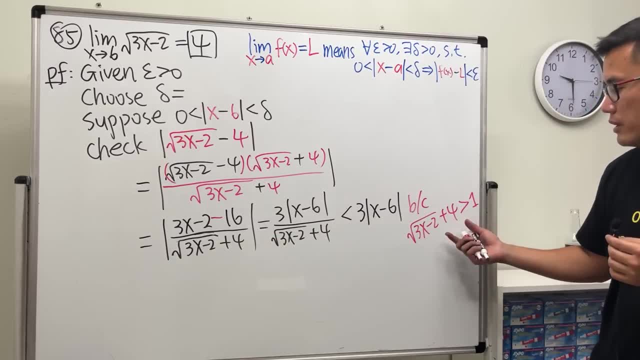 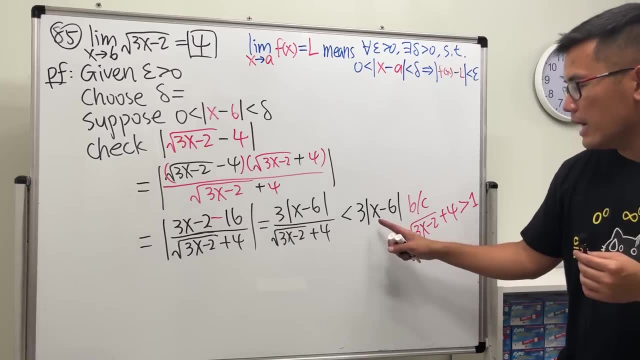 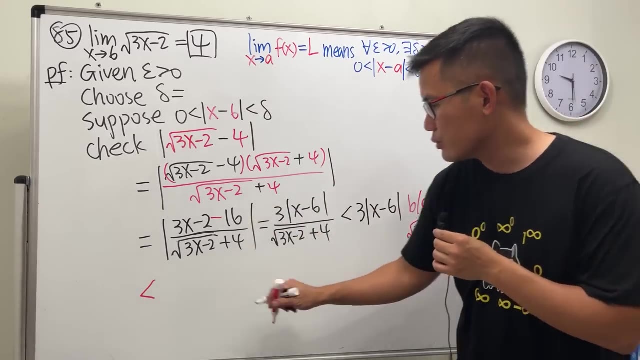 absolute value, but from here to here, we mention this is greater than 1 because we want to have this inequality and get rid of the whole thing. cool, now we have this, which is that which is excellent. so this right, here it's again another less than thanks to that and we have a 3 right. 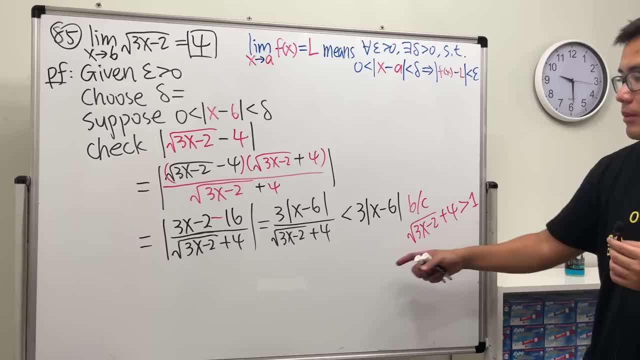 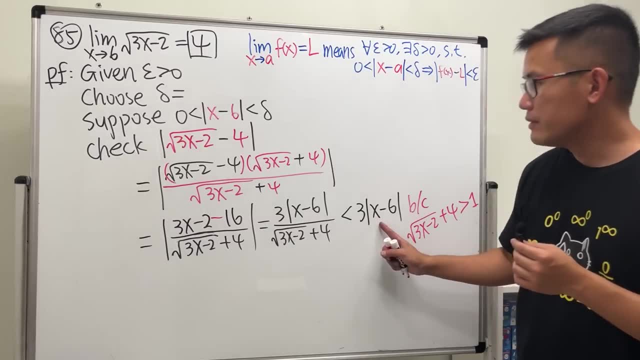 But from here to here we mention this is greater than 1, because we want to have this inequality and then get rid of the whole thing. Cool, Now we have this, which is that which is excellent. So this right here is again another less than. 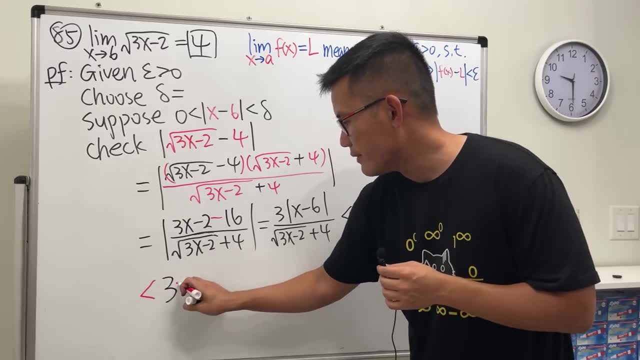 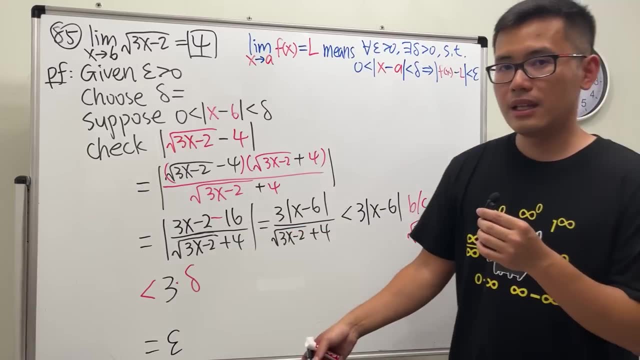 Thanks to that and we have a 3 right here. And then we have a delta, And we know it. At the end we want to have just epsilon. So now, what's the delta? Epsilon over 3.. 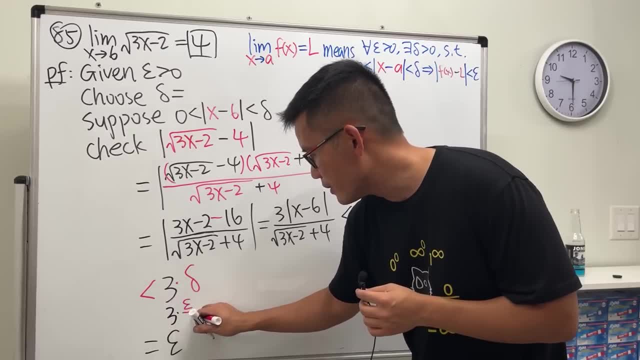 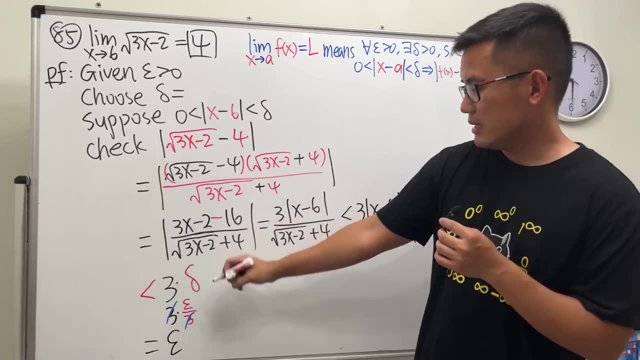 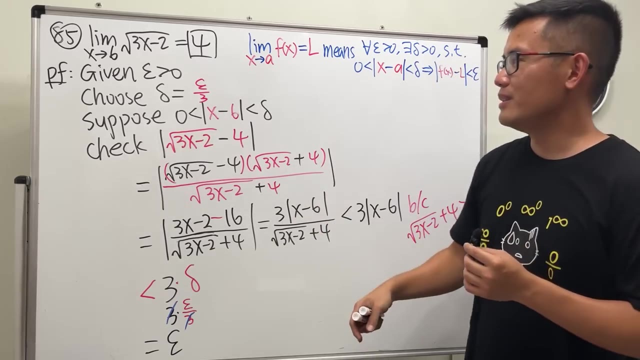 Yes, this is 3 times Epsilon over 3.. And then we have this and that Bye-bye. So we come back here and then say delta is equal to epsilon over 3.. This is so cool. This is symmetric if you rotate 180 degrees. 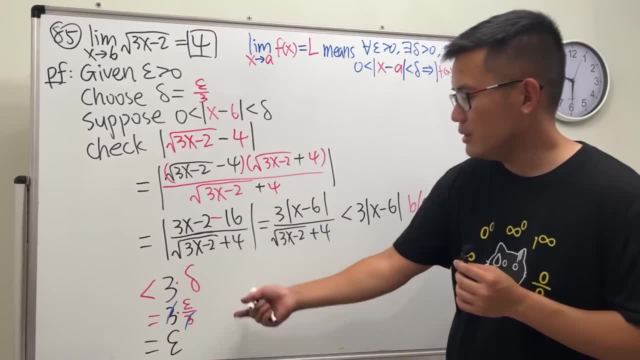 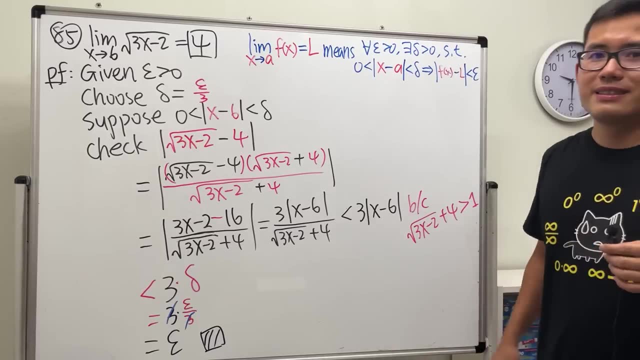 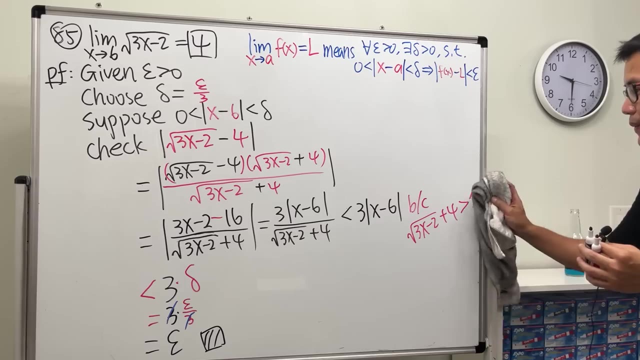 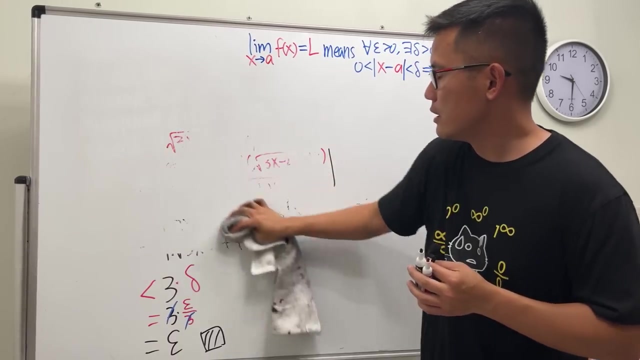 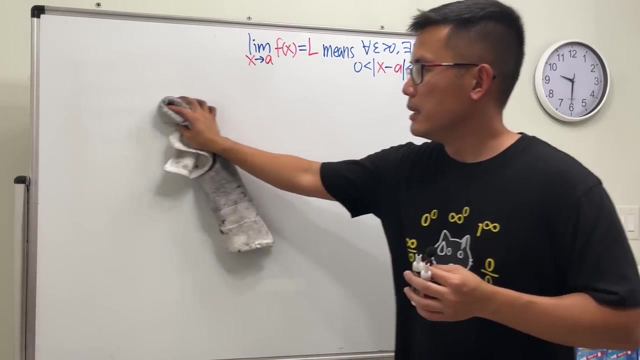 Yeah, Anyway, this is equal. Delta is equal to epsilon over 3.. And then we are done, We're done, Done, Yeah, We're done, Yeah. No, We have a couple more to go, of course, Alright. 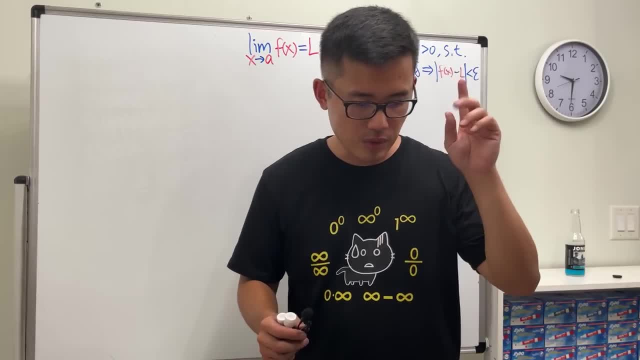 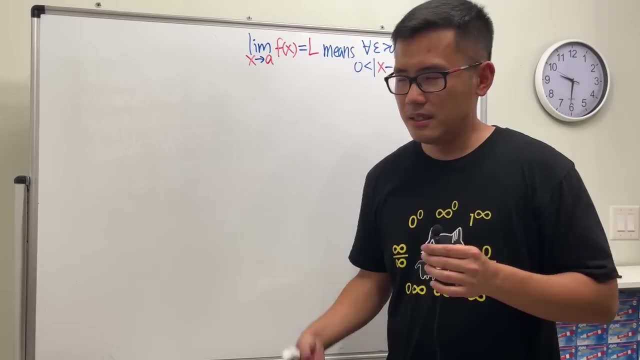 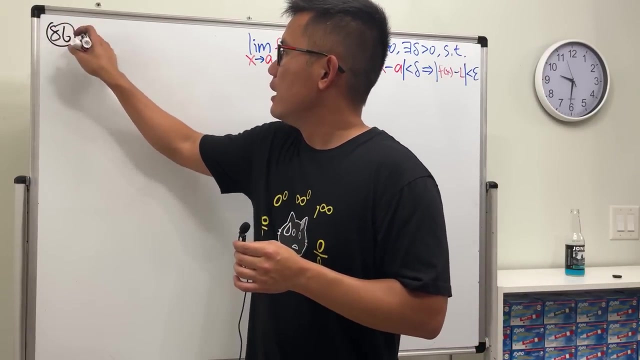 Quadrantic cases. So two quadratic cases And then one cubic And then two rational, And then we'll move on to Riemann's sum And it will be done. Alright, Number 86. Limit: as x approaching, We have 3.. 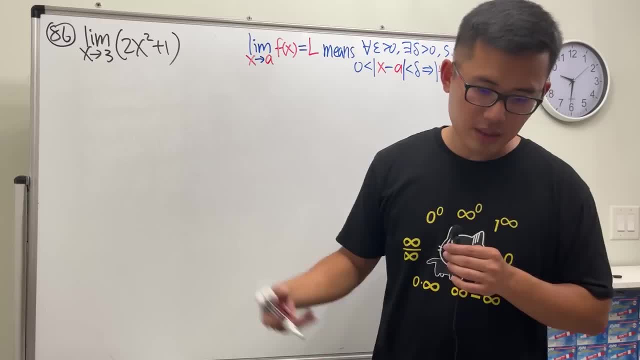 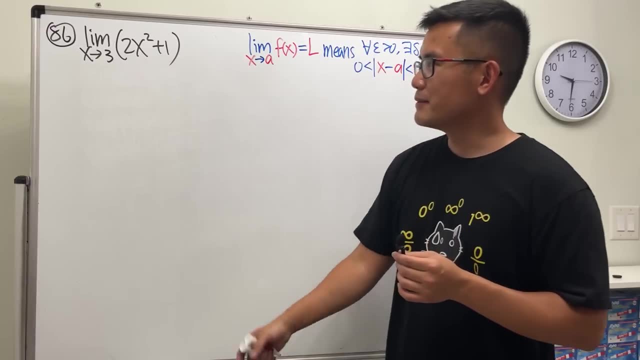 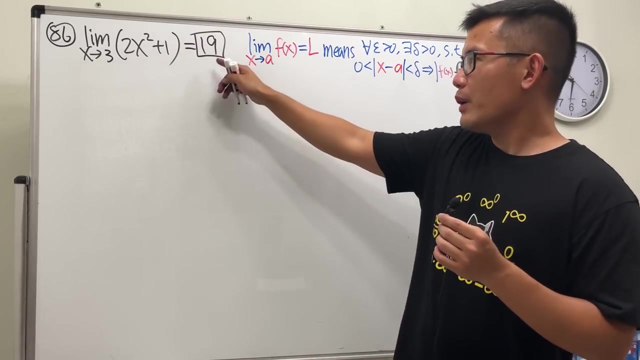 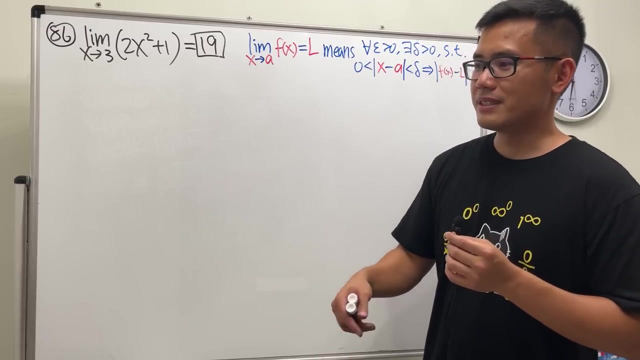 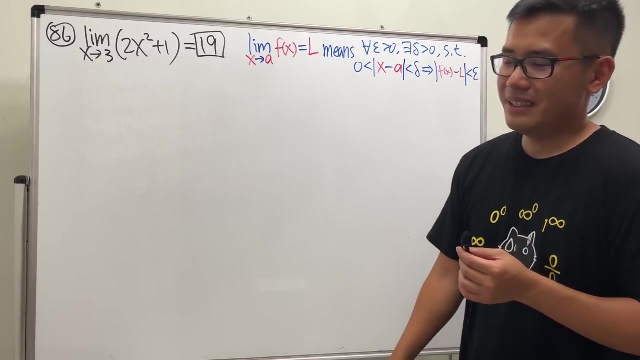 2x squared plus 1.. Let's just work this out real quick: 3 squared is 9.. 11,3.. Alright, Remember we already did 1.. We don't have the. I don't know Anyway. 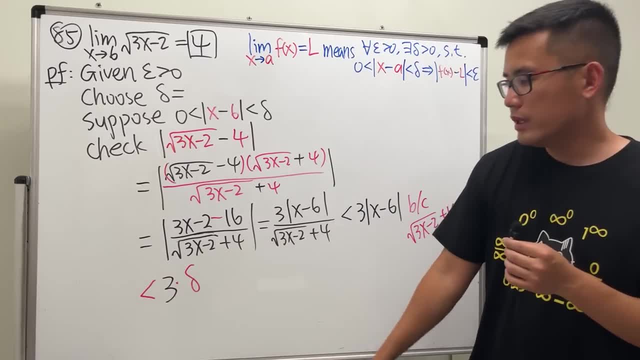 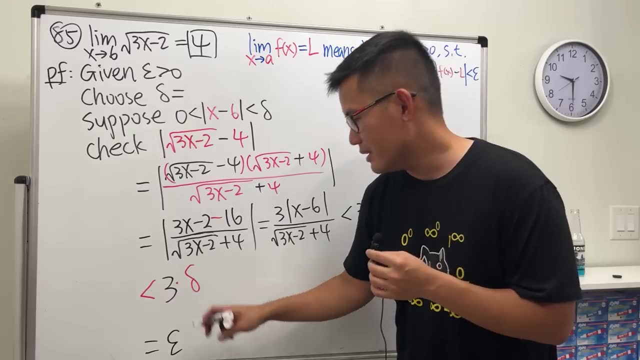 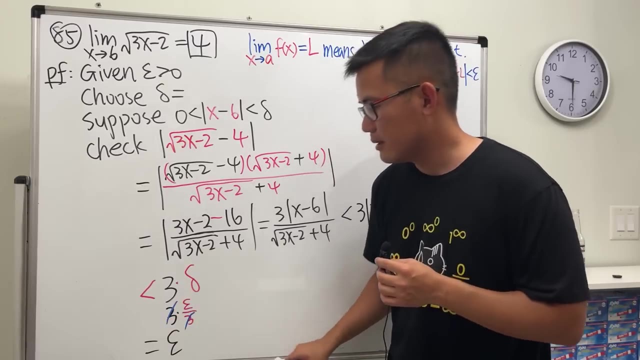 here, and then we have a delta, and we know it, at the end we want to have just epsilon. so now, what's the delta? epsilon over 3, yes, this is 3 times epsilon over 3. and then we have this and that, bye, bye. so we come back here and then say: 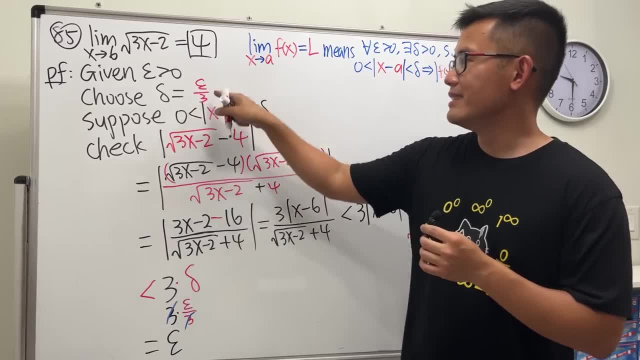 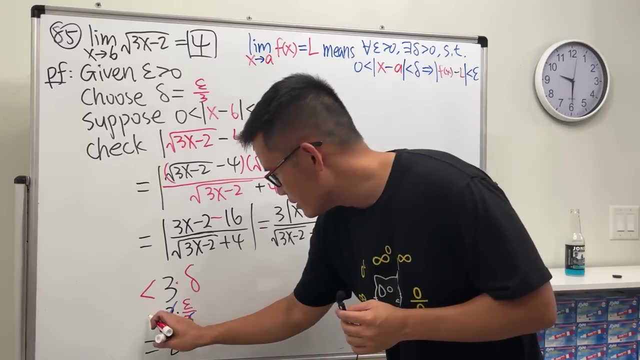 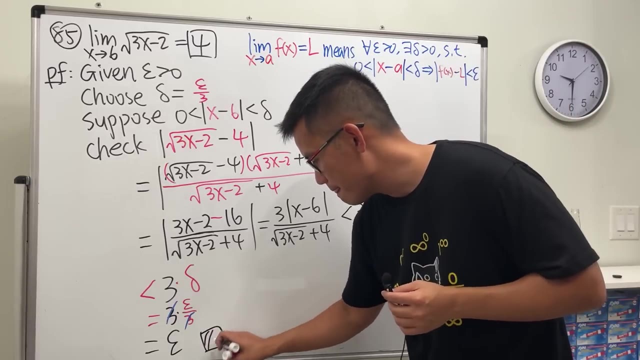 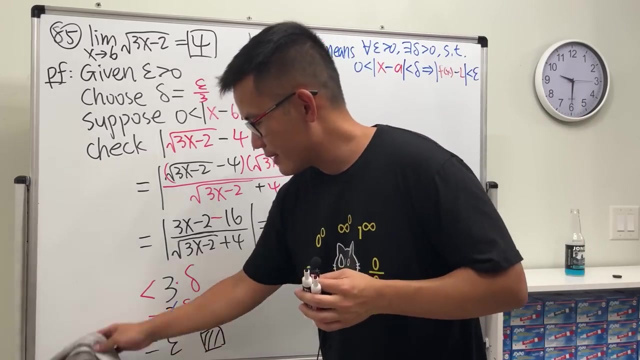 delta is equal to epsilon over 3. this is so cool. this is symmetric. if you rotate 180 degrees, yeah, anyway, this is equal. delta is equal to epsilon over 3, and then we are done, we're done, done, yeah right, yeah, yeah. no, we have a couple more to go, of course. 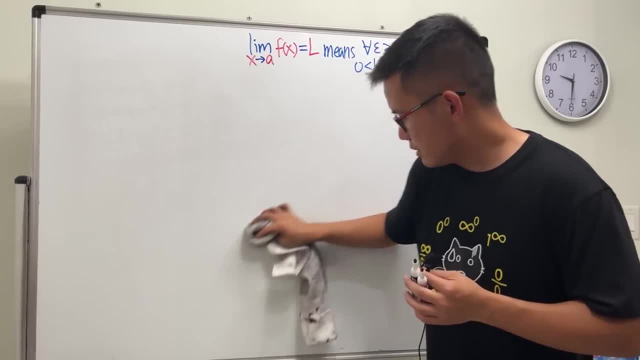 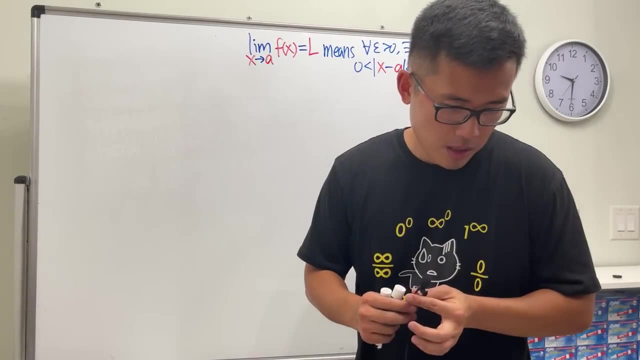 squadron t cases. so to quadrometry cases. so two quadratical cases, the joules x and the two exploded cases. the velocity units goes up two times ические cases. one will not be the homogeneity case, one will not get the simple functions, yours and 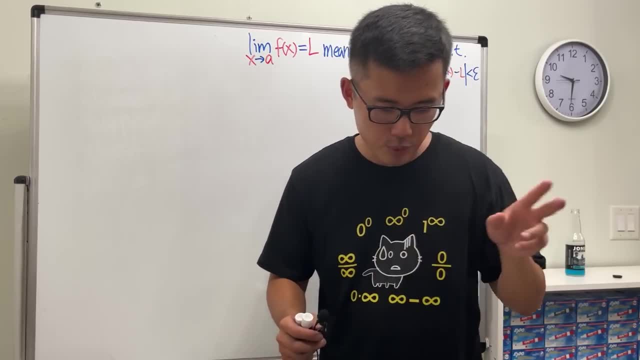 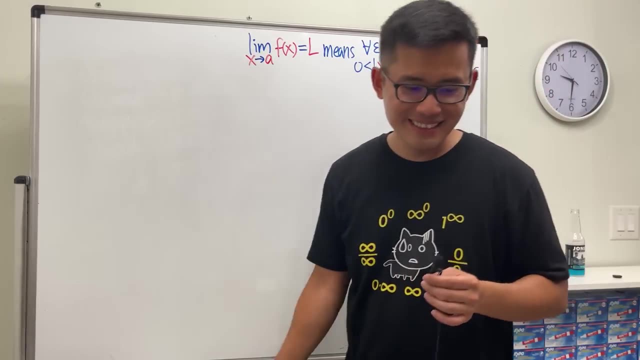 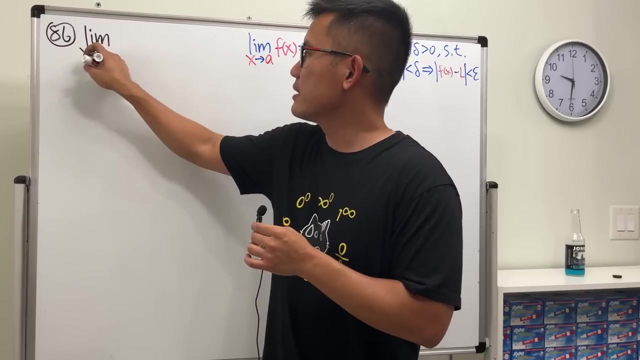 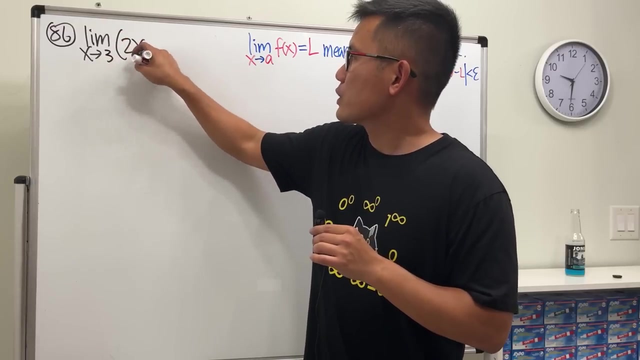 quadratic cases, and then one cubic, and then two rational, and then we'll move on to Riemann's sum and it will be done all right. number 86 limit as x approaching, we have three, two x square plus one. let's just work this out real quick. three square is nine. 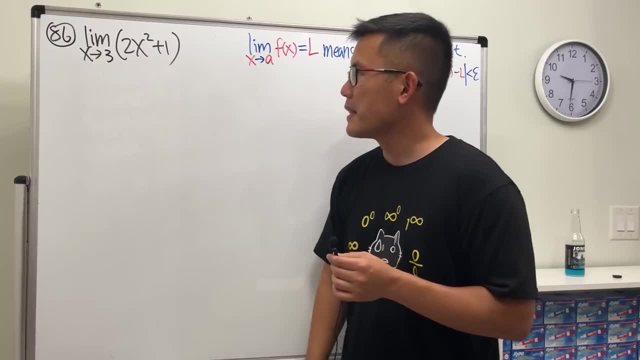 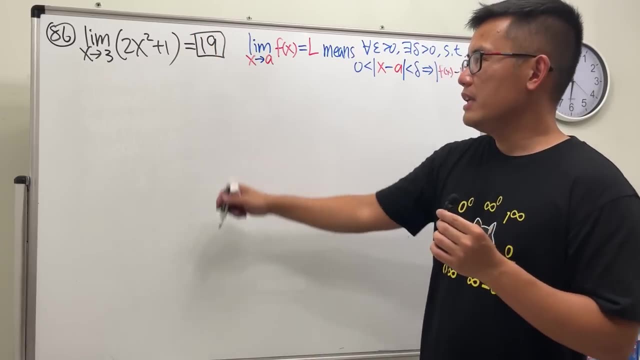 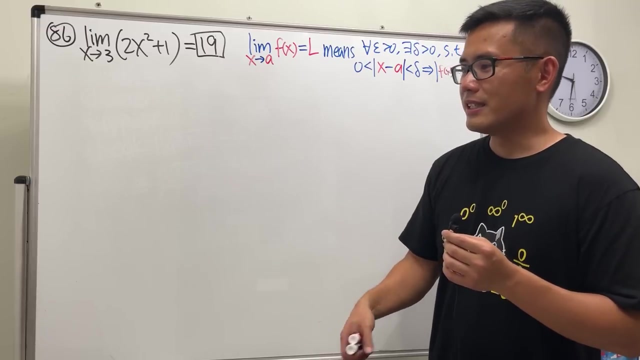 times two is 18 plus one is 19. all right, here's the deal. if somehow you computed this wrong, let me tell you later on. the proof is going to horrendous if the proof does not go as smooth as the example that i've been showing you. 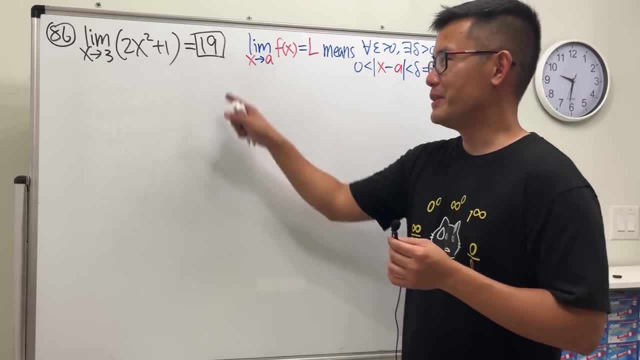 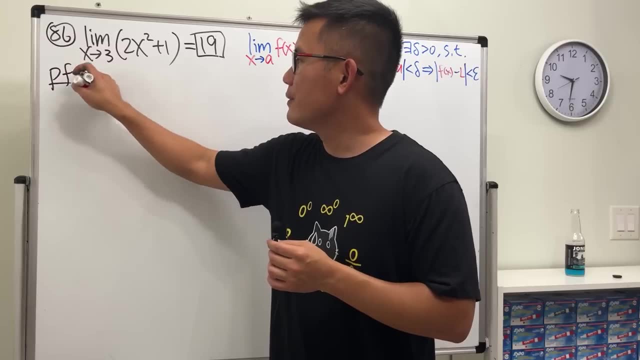 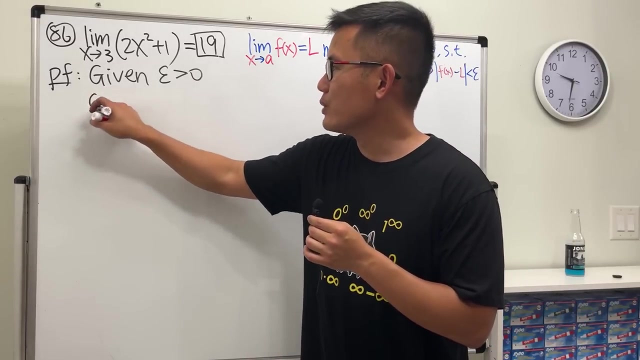 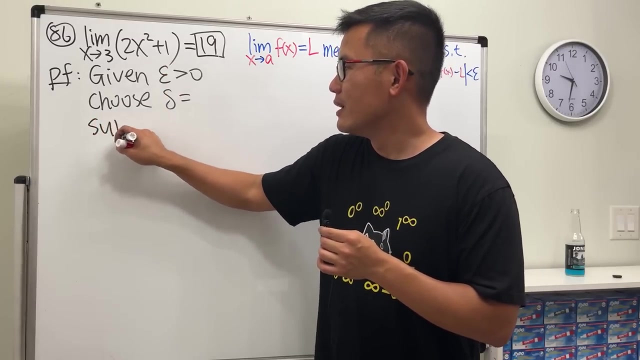 earlier. maybe we just actually did something wrong in the beginning, i don't know. anyway. pf proof given epsilon greater than zero. and then we are going to choose delta- i don't know yet, but you know i'm not worried about it- suppose epsilon value x minus three. 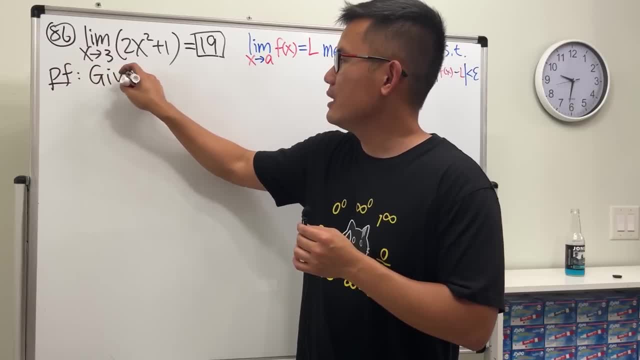 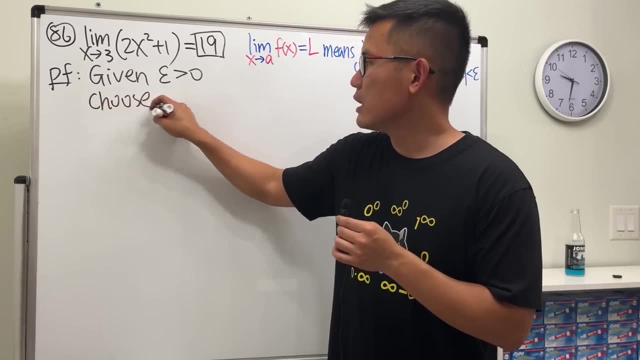 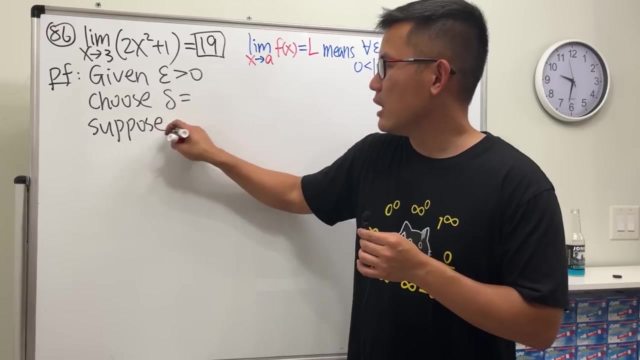 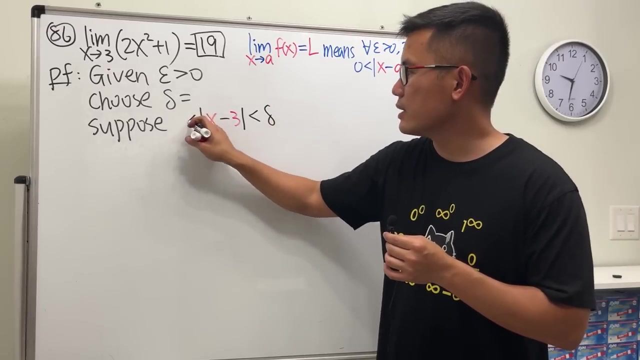 We're done. So we're done. We're done. have proof given epsilon greater than 0, and then we are going to choose delta. i don't know yet, but you know i'm not worried about it. suppose epsilon value x minus 3 is less than delta and then not greater than 0, like this. lastly, we are going to check and 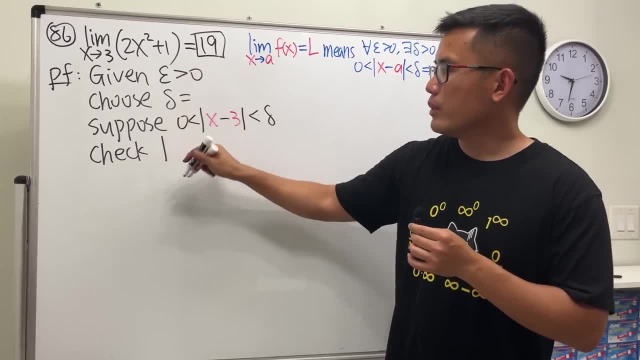 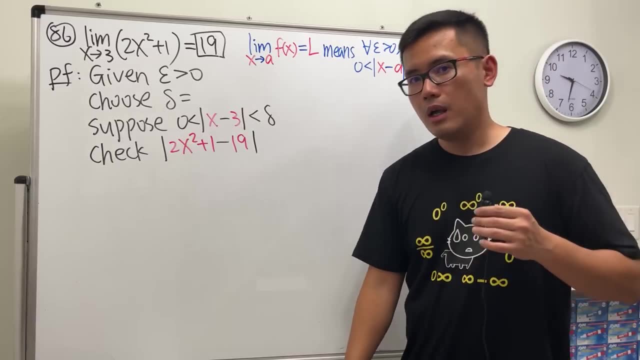 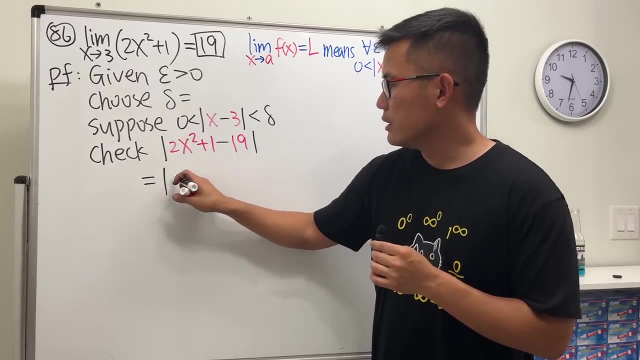 hopefully everything goes smoothly. absolute value of the function: 2x squared plus 1, minus the limit, which is 19. all right, here we go. this minus die is minus 18, and then we can factor out 2, so this right here is 2. all right, let's see. all right, 2x squared. 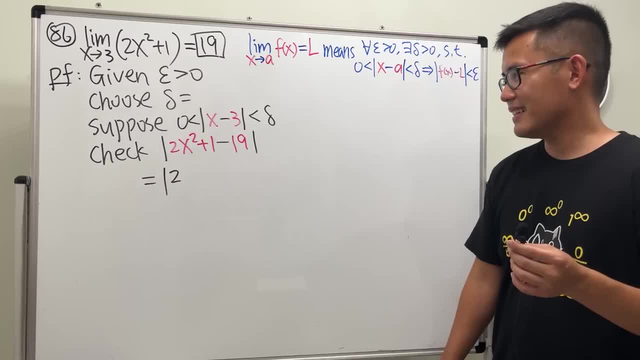 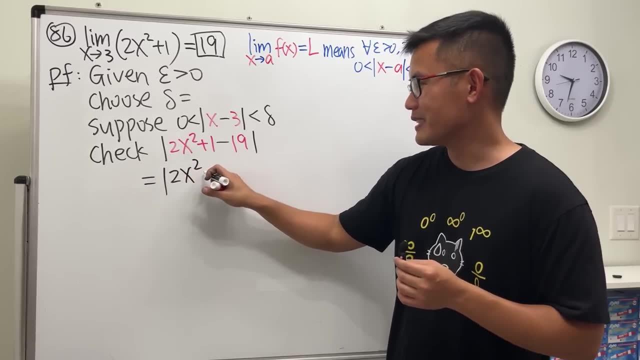 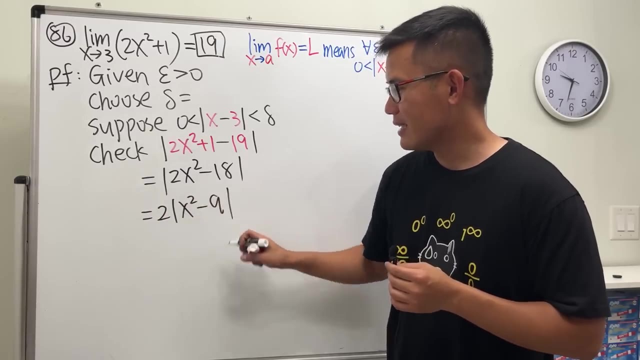 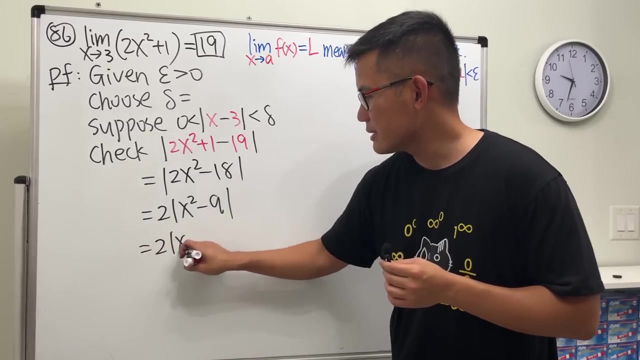 hold on, okay, okay, okay, okay. 2x squared- i'll show you guys all the steps: minus 18, and then we factor out 2, and then we get x squared minus 9. all right, and perhaps i'll: yeah, yeah, this is okay, and then okay, and then this is: 2 times x minus 3 times x plus 3. 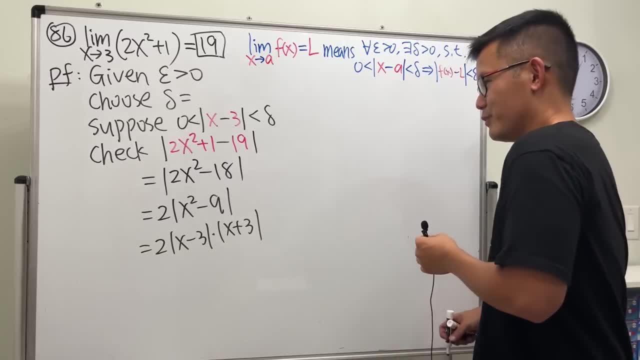 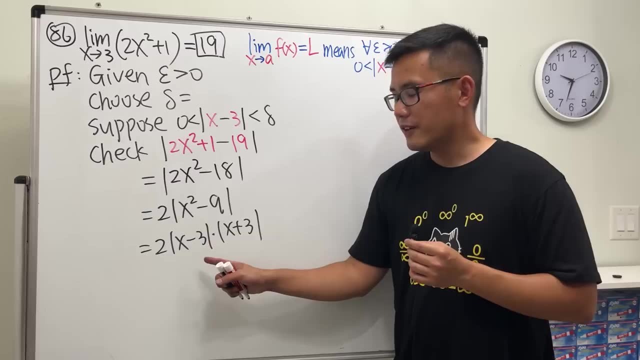 okay, so show all the steps more legitimate. i was going to go from here to here, but no, yeah, sure you. you guess everything. and from here to here we use the fact that the absolute value of a product is the product of the absolute value. so it's pretty clear, so you can skip that. 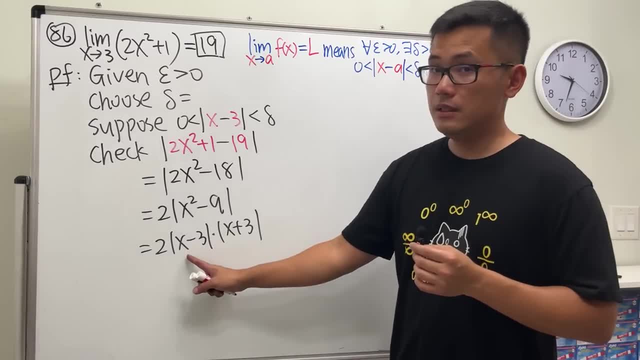 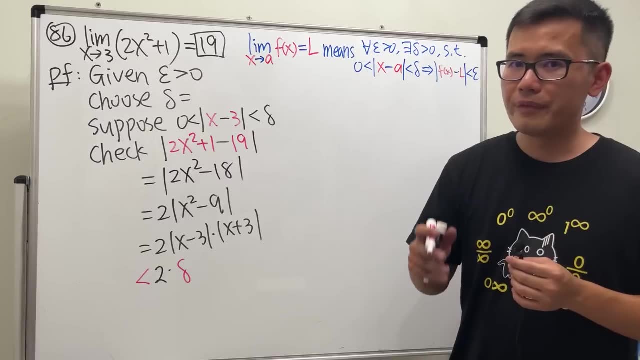 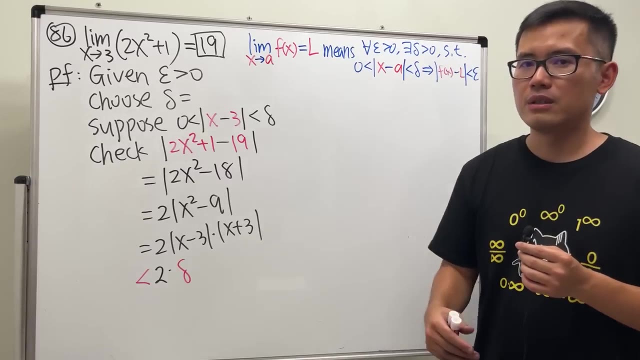 it's another step, but anyway, though, this is nice because we can say that we can have less than 2 times delta. but now here's the troublesome absolute value of x minus 3. how can we get rid of it? well, how can we get a bound? meaning that we want to show this right here is less than some number. 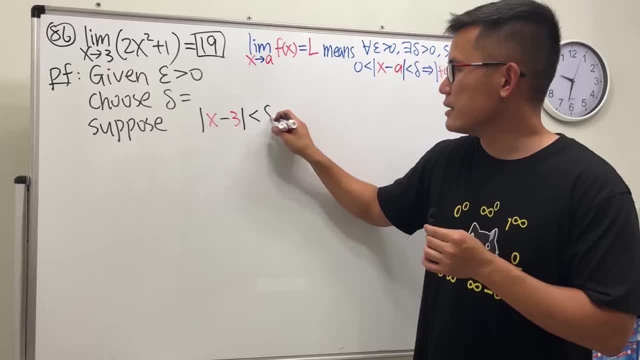 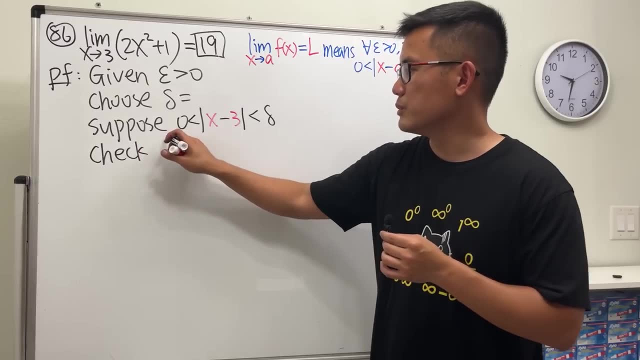 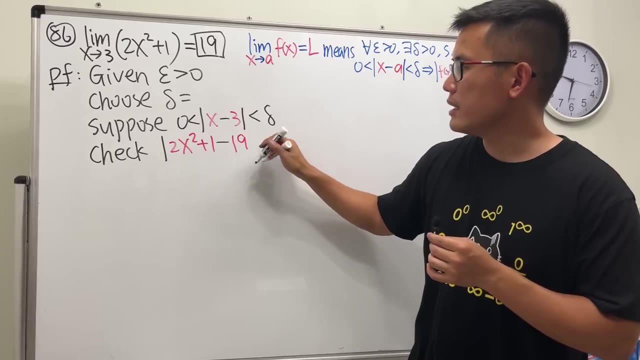 is less than x minus three delta, and then not greater than zero, like this. lastly, we are going to check, and hopefully everything goes smoothly: absolute value of the function 2x squared plus one, minus the limit, which is 19. all right, here we go, this minus. 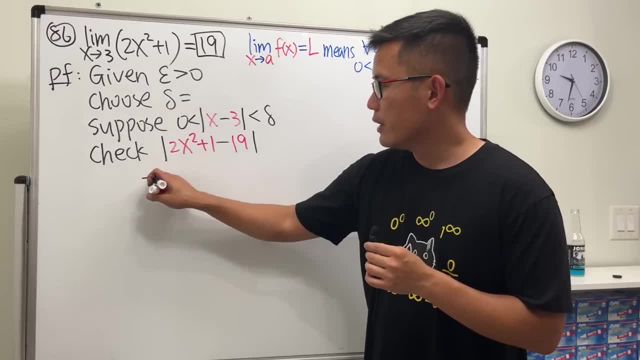 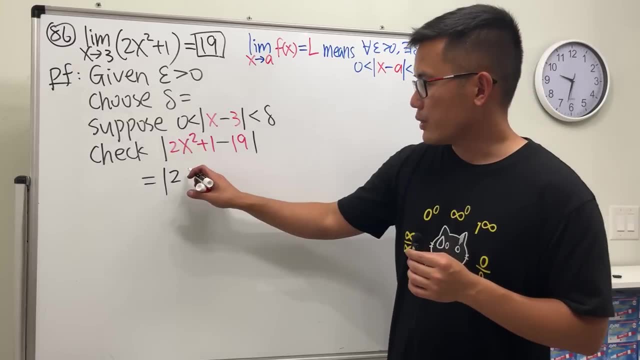 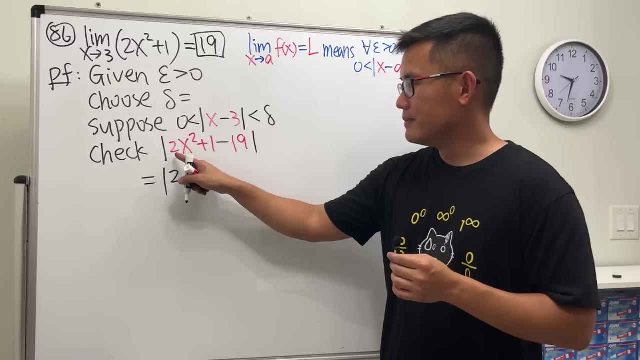 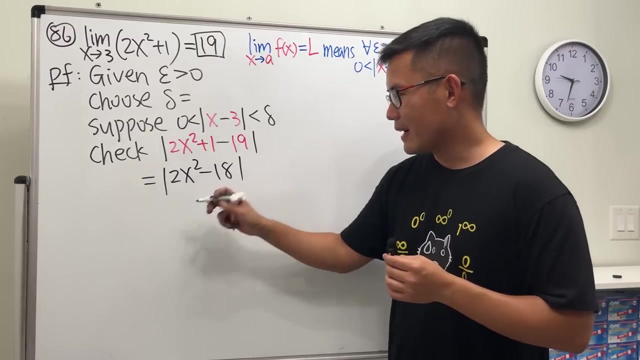 die is minus 18, and then we can factor out two. so this right here is two. all right, let's see. all right, 2x squared, 2x squared. I'll show you guys all the steps: Minus 18, And then we factor out 2. 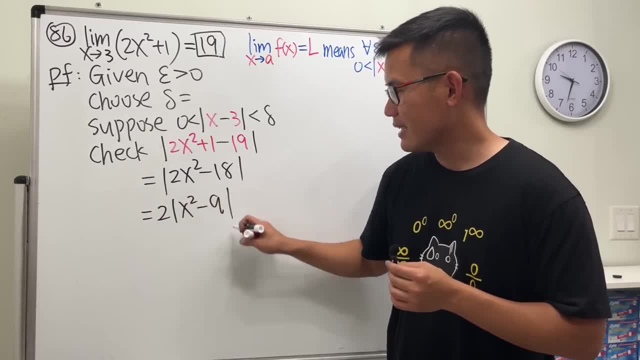 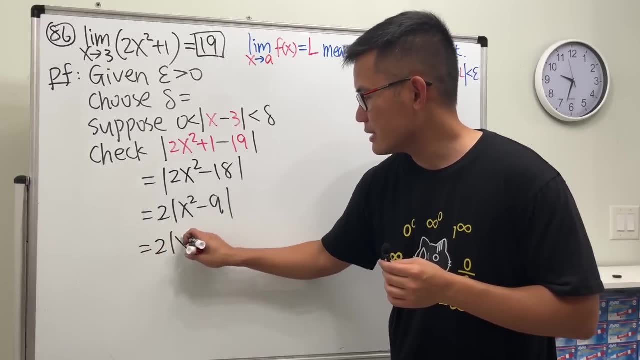 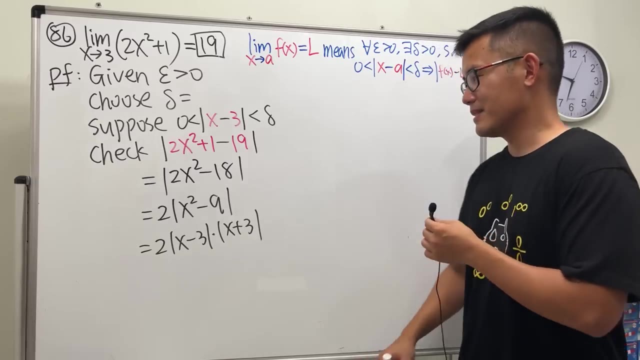 And then we get x squared minus 9. Alright, and perhaps I'll. Yeah, yeah, this is okay. And then, And then, this is 2 times x minus 3, Times x plus 3. Okay, so Show all the steps. I was going to go from here to here, but 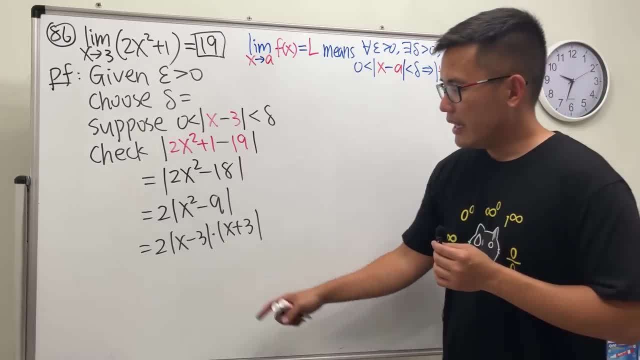 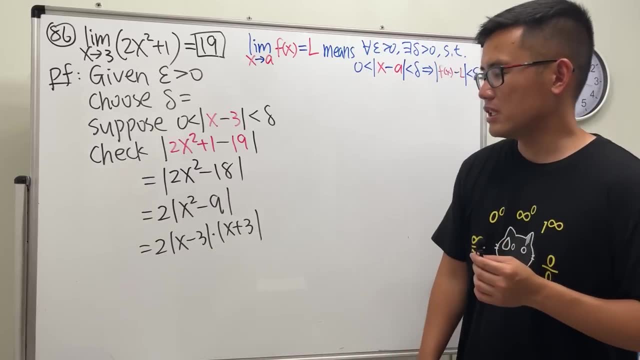 No, yeah, I'll show you guys everything. And from here to here We use the fact that the absolute value of a product Is the product of the absolute value. So it's pretty clear. so you can skip that. It's another step, But anyway, though. 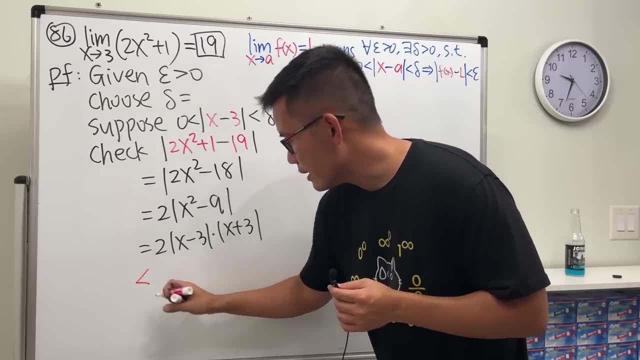 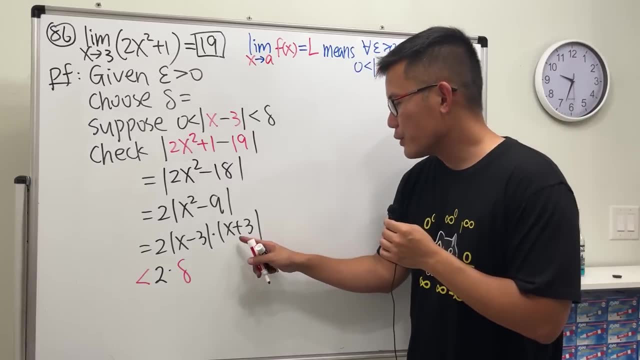 This is nice because we can say that We can have less than 2 times delta. But now here's the trouble: Absolute value of x minus 3. How can we get rid of it? Or how can we get bound Meaning that We want to show? 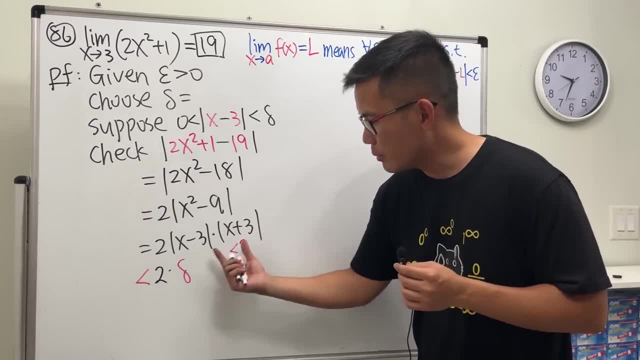 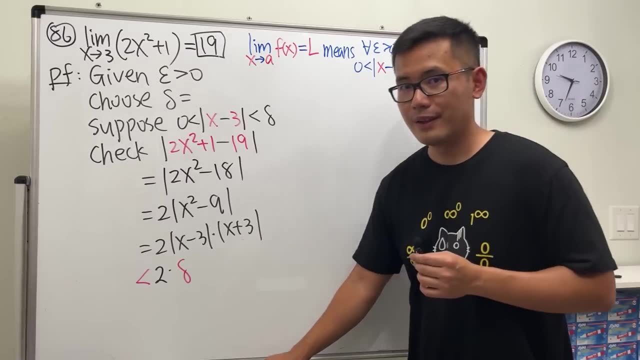 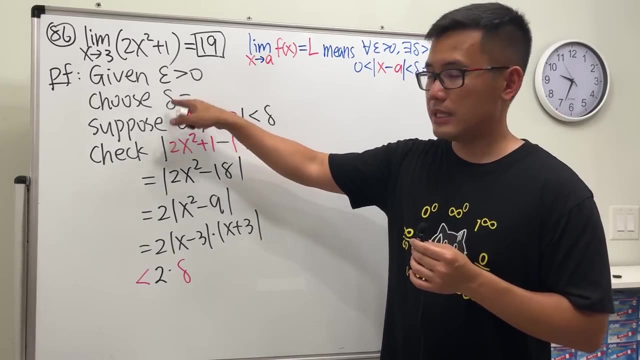 This right here is less than some number as well, So that we can kind of maintain this inequality, So it can go smoothly. How do we do it though? Okay, This is where the magic is. We are going to come back to the delta. Come back here right now. 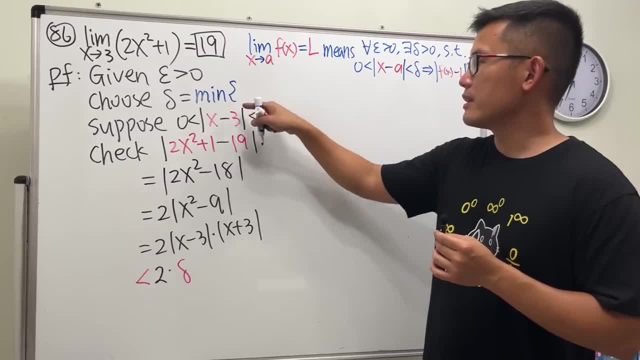 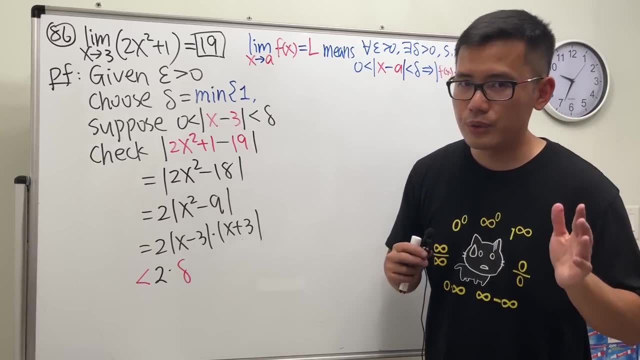 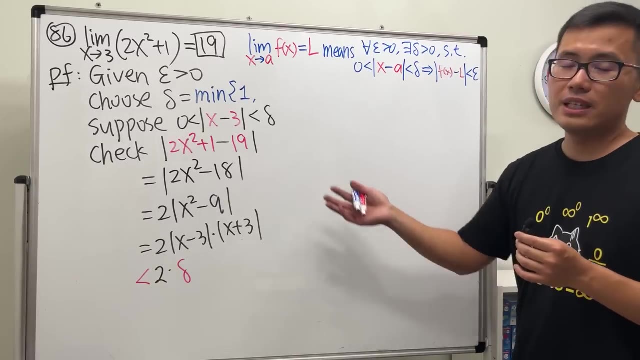 And then put down minimum, And then like this notation, Like set notation, And then just use one. Keep in mind: just use one. Oh, I heard. can you use two? Can you use seventeen? Sure, up to you. If you want to have a smooth experience, Then I highly recommend you to use one. 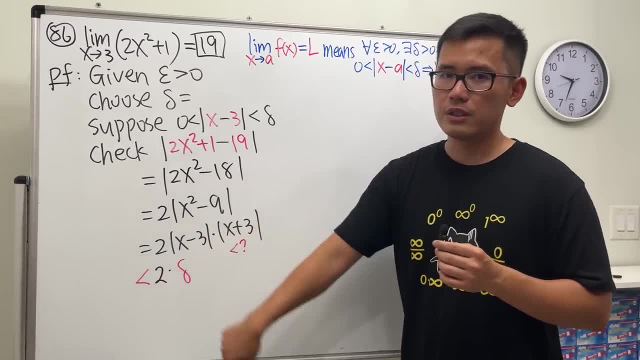 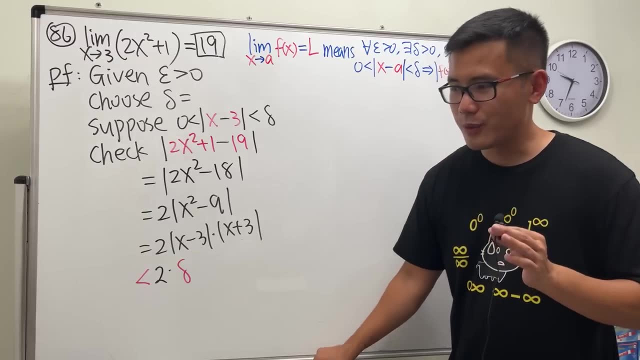 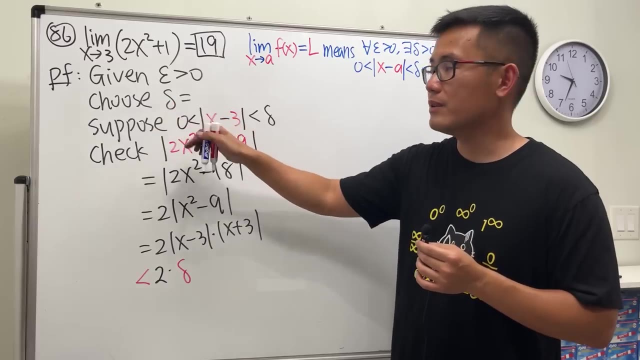 less than some number as well, so that we can kind of maintain this inequality, so it can go smoothly. uh, how do we do it though? okay, this is where the magic is. we are going to come back to the delta, come back here right now, and then put down minimum, and then like this notation, like: 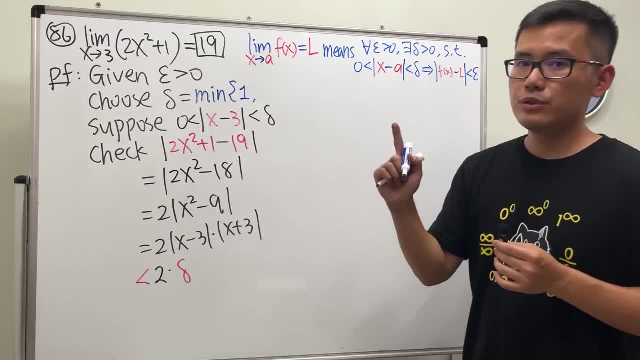 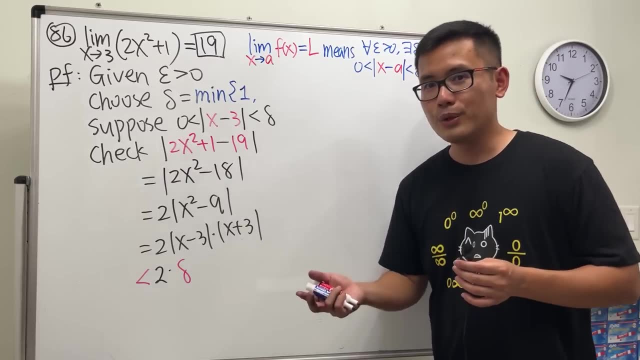 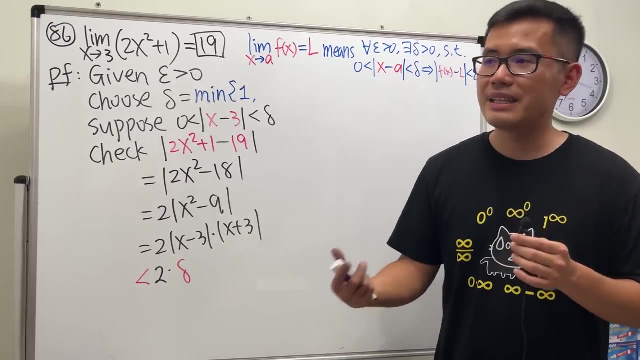 set notation and then just use one. keep in mind, just use one. oh, i heard, can you use two? can you use 17.. sure, up to you. if you want to have a smooth experience, then i highly recommend you to use one. if you want to have some at at um adventures, use pi. use one over e. 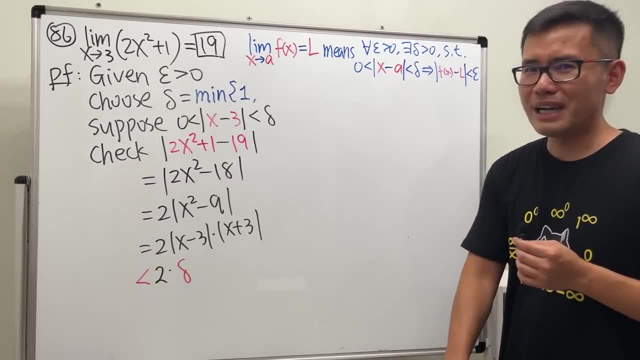 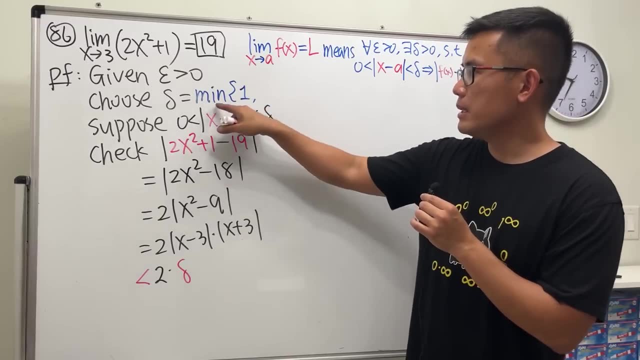 just use one, please. no, no, use one over pi. sometimes too, yeah, i don't know, but anyway, just put on one. why? because the moment that we have the minimum and also the one, the moment that we have the minimum and also the one, the moment that we have the one right here, we are allowed to come here and say: 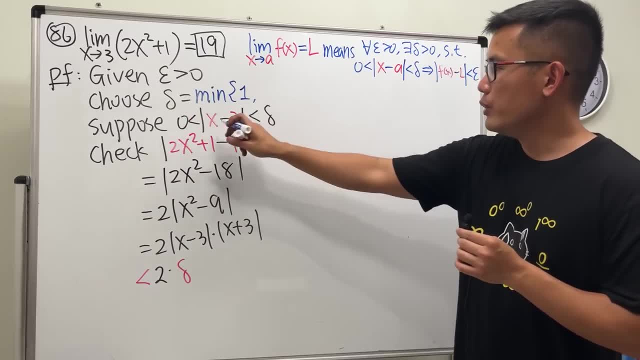 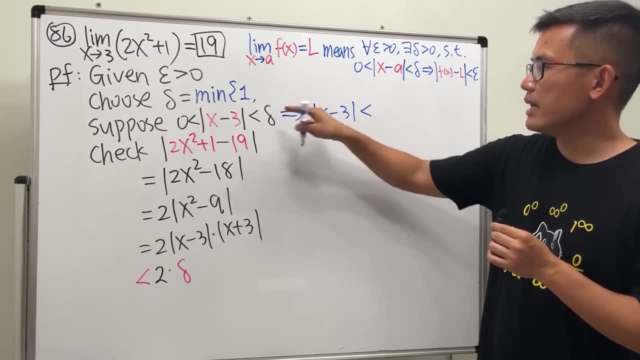 because, delta, we have this one that we can use. so look at this equality, just this side, and we can say: absolute value of x minus three is less than this number that we put down earlier. we put down one so we can use one. we put down one over e. 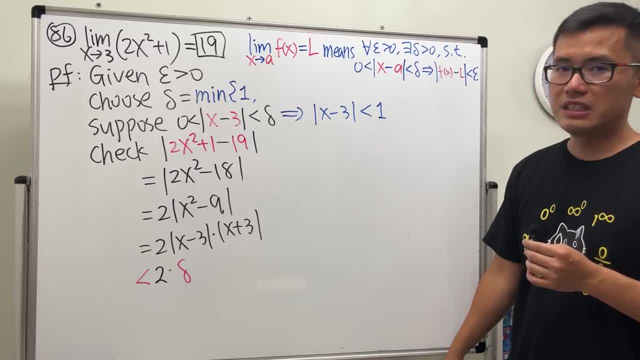 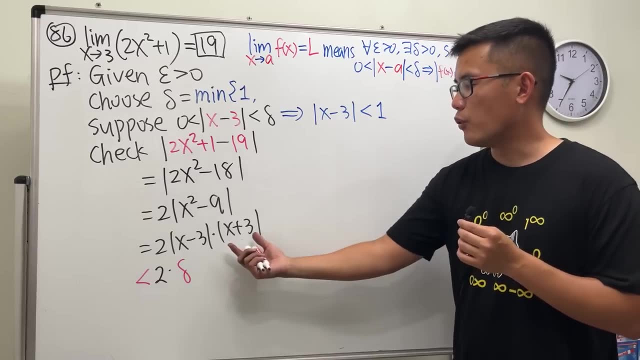 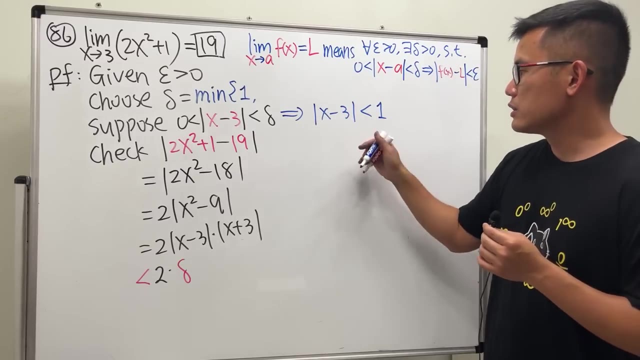 you use one over e. you want to put on square root 17, square root 17. up to you. now, from here, we are going to somehow get an expression for absolute value of x plus three. to do so one systematic way is just: you first open the absolute value. so we will. 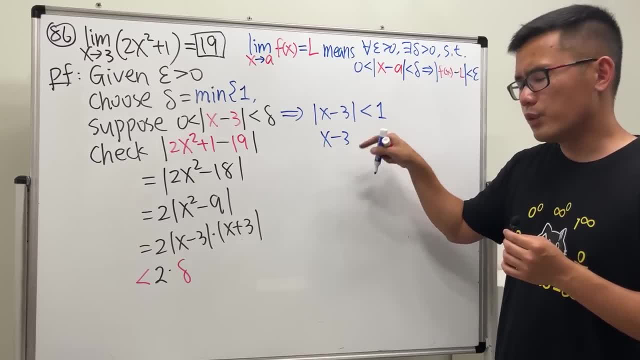 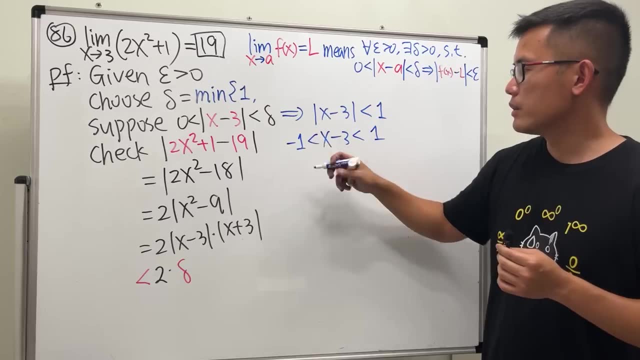 know that when we do that, we get absolute value. we will get x minus three. this right here will be in between of one and negative one, right? that's how absolutely works, right? if this is less than one, then that means the inside is in between of negative one. 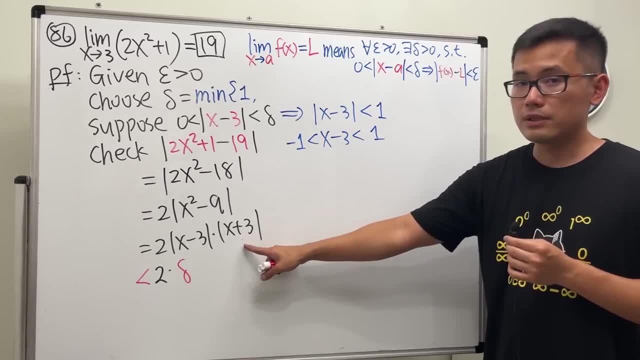 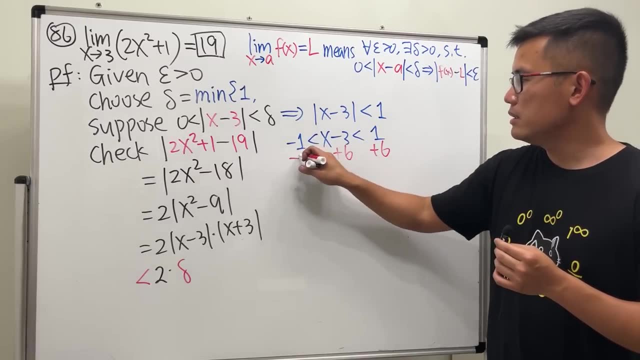 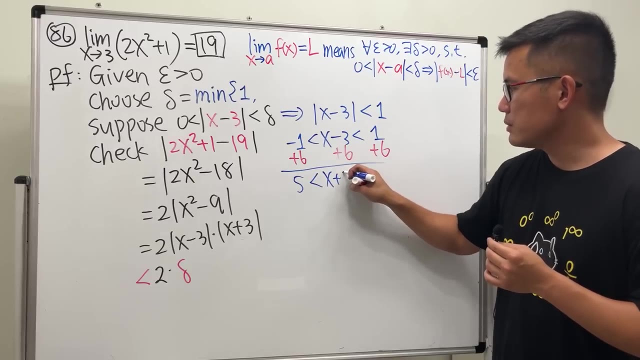 and one, and now you see we want to have x plus three. this is x minus three, so let's just go ahead and add six to everybody, and this is of course legitimate, because this is just a regular inequality. and then you see, this is five and this is x plus. 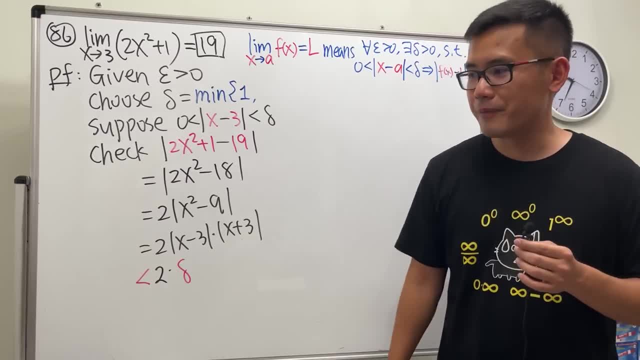 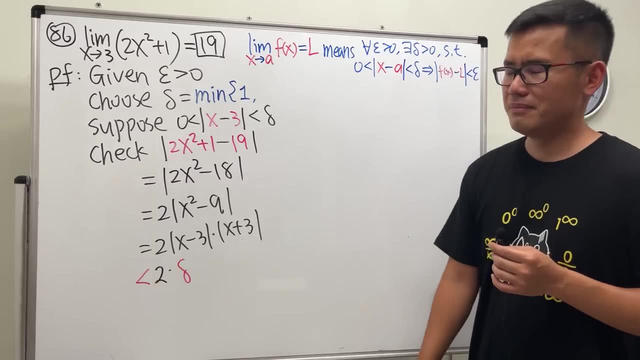 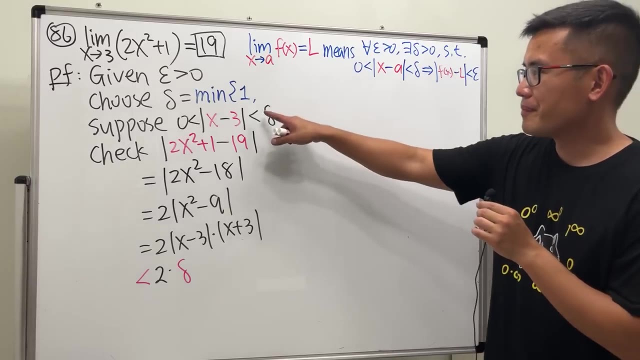 If you want to have some adventures, Use pi, Use one over E. Just use one, please. No, no, no, use one over pi. sometimes too, Yeah, yeah, I don't know, but anyway, just put on one. why? because the moment that we have the minimum and also the one, the 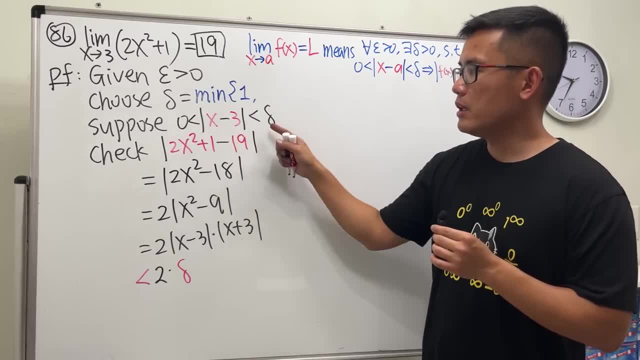 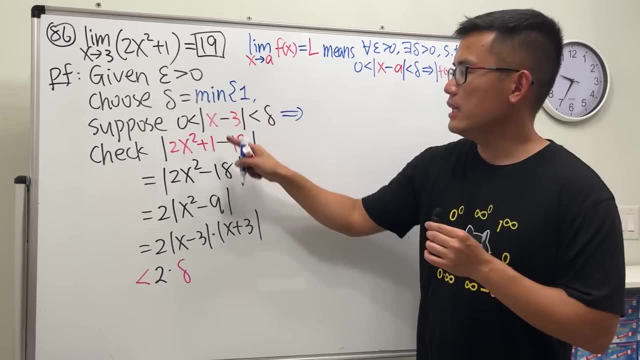 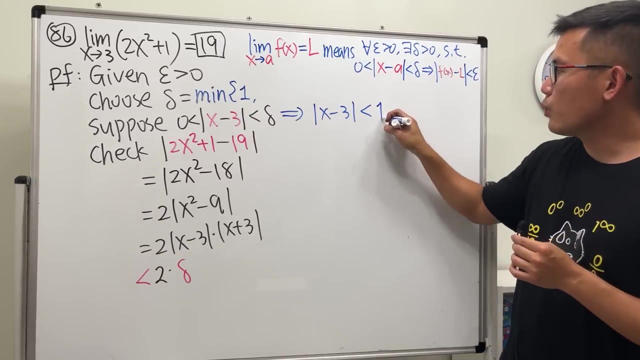 moment that we have the one right here, we are allowed to come here and say: because, delta, we have this one that we can use. so look at this equality, just this side, and we can say: absolute value of x minus three is less than this number that we put down earlier. we put on one, so we can. 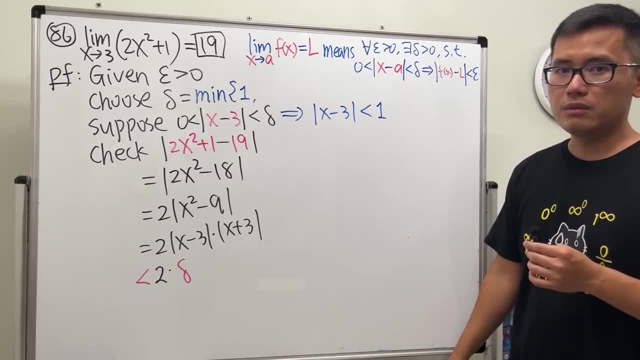 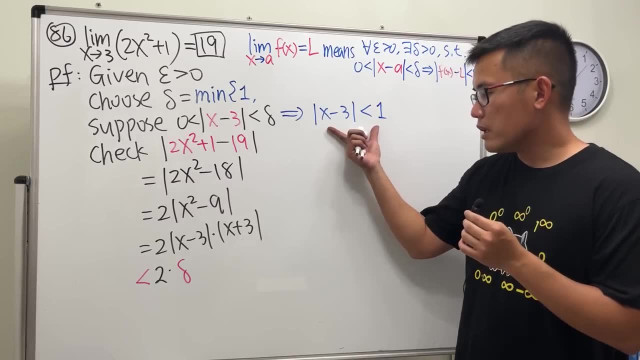 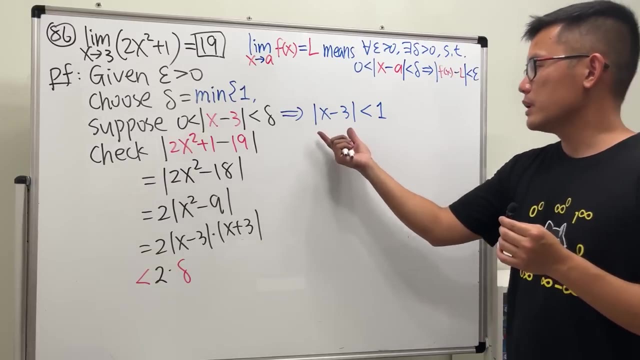 use one. we put on one over e. you use one over e. you want to put on square root 17. square root 17. up to you. now, from here, we are going to somehow get an expression for absolute value of x plus three. to do so one systematic way is just you first open the absolute value, so we will know that. 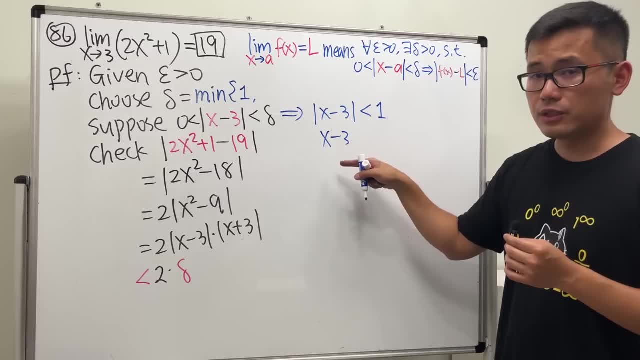 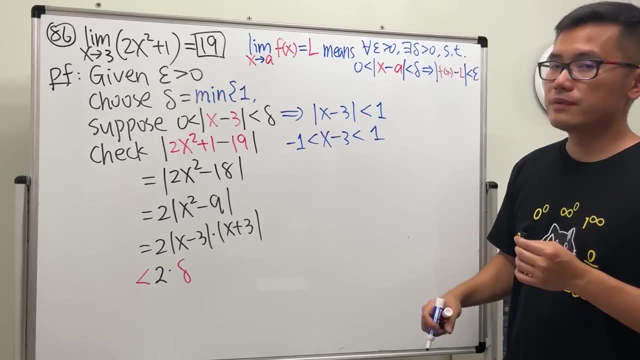 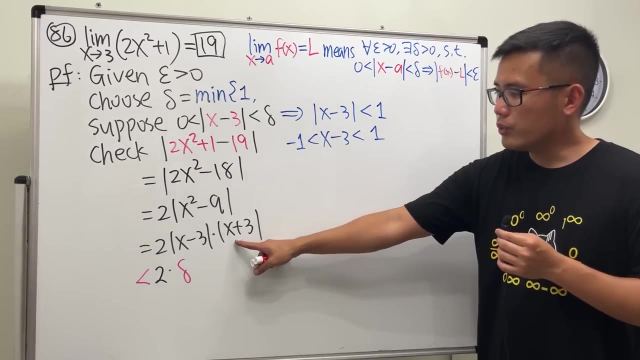 when we do that, we get absolute value. we get x minus three. this right here will be in between of one and negative one, right? that's how absolute value works, right? if this is less than one, then that means the inside is in between of negative one and one. and now you see, we want to have x plus three. this is x minus. 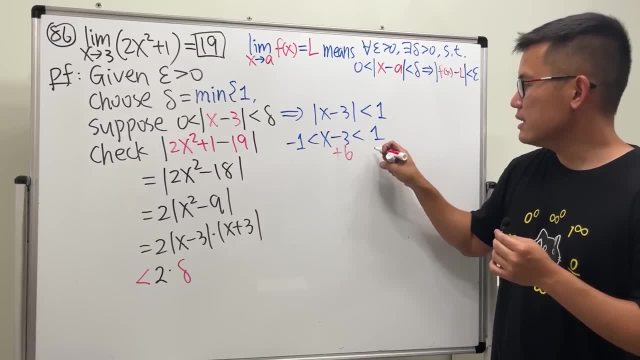 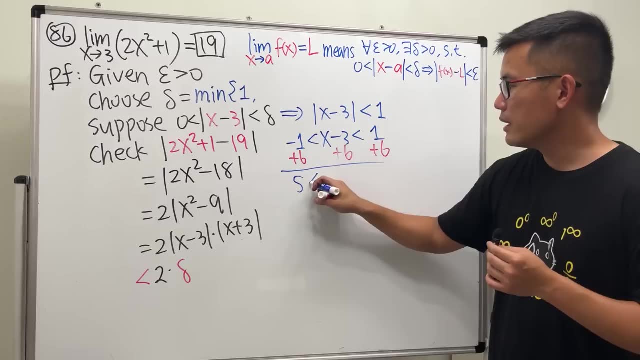 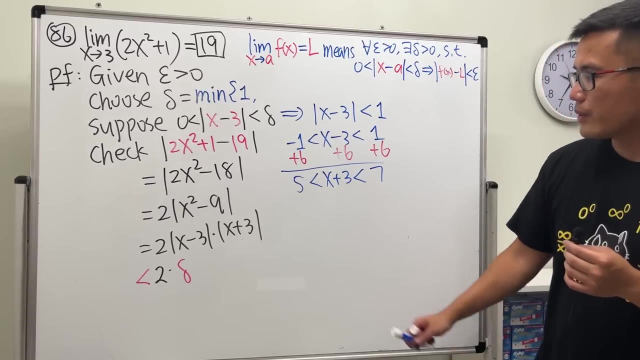 three. so let's just go ahead and add six to everybody, and this is of course legitimate, because this is just a regular inequality- and then you see this is five, and this is x plus three, and then this is seven. okay, now question for you guys. i want to go from here back to the absolute value. how do we do it? 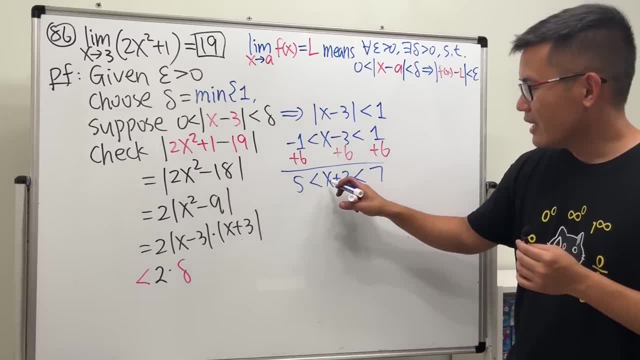 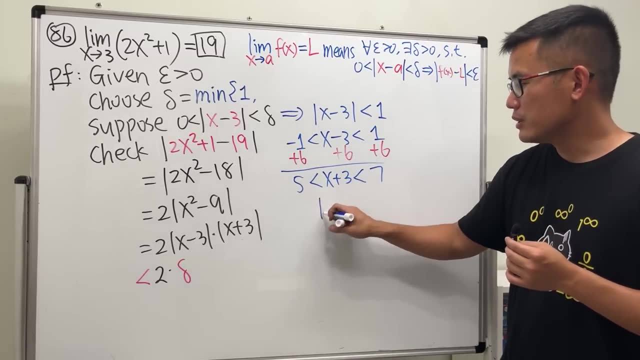 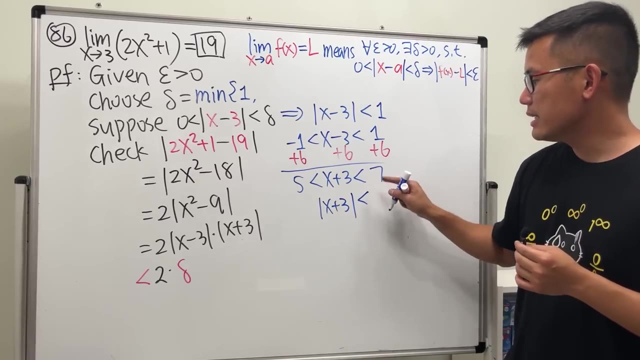 well, here's the idea. just compare the absolute value of this number and the number. which one is bigger. seven has a bigger absolute value, so it's just absolute value of x minus x plus three. absolute value of x plus three is less than this number, the bigger absolute value. why? because when 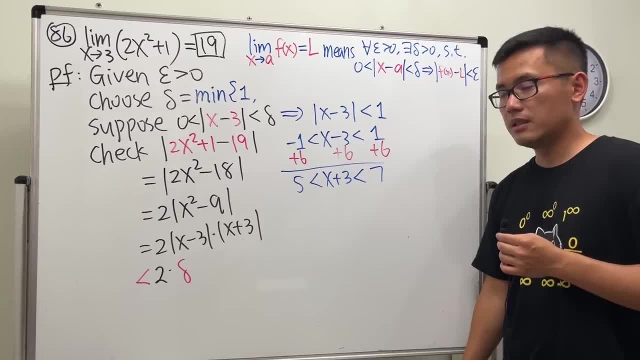 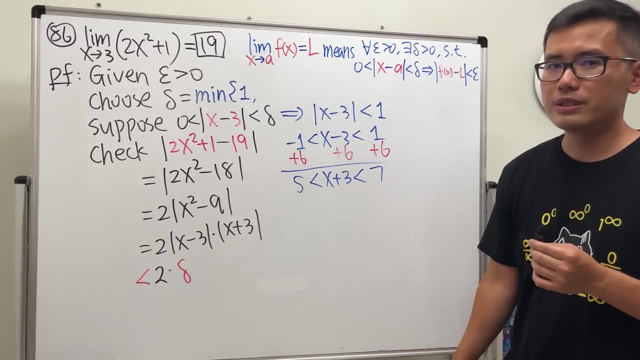 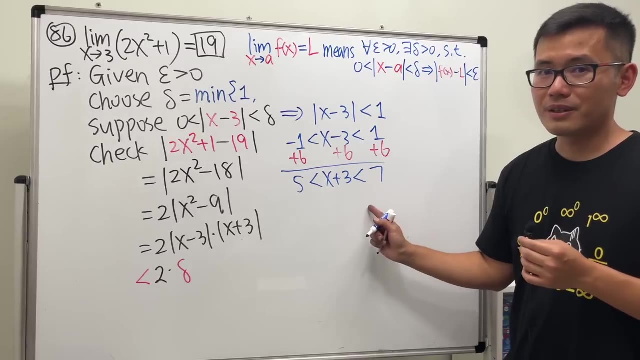 three, and then this is seven. okay, now question for you guys. i want to go from here back to the absolute value. how do we do it? well, here's the idea: just compare the absolute value of this number and the number. which one is bigger. seven has the bigger absolute value, so it's just absolute value of x. 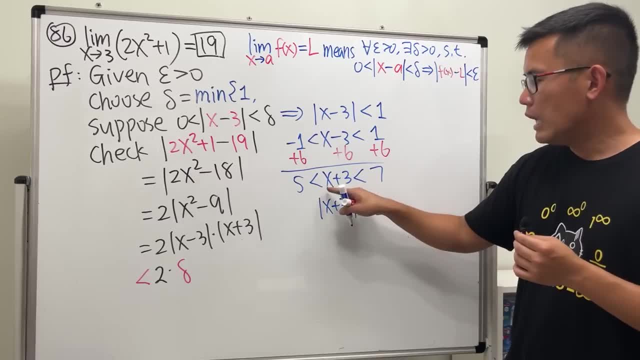 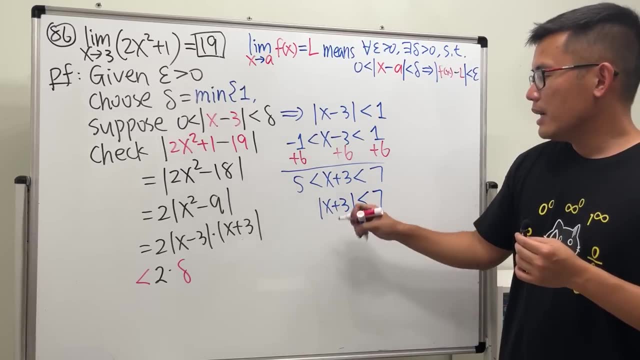 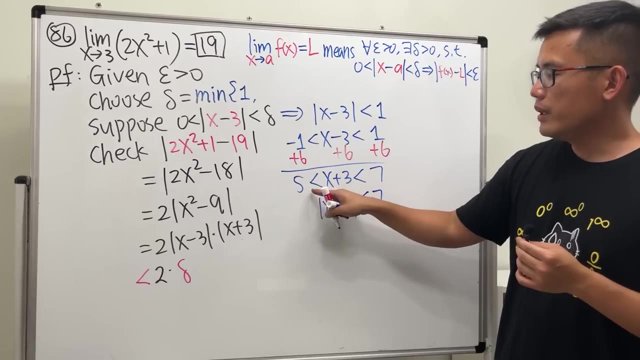 minus x plus three. absolute value of x plus three is less than this number, the bigger absolute value. why? because when we have this, of course, x plus three, if it's greater than five, it has to be greater than negative seven. so you see that we have negative seven, also seven, so of course we can write. 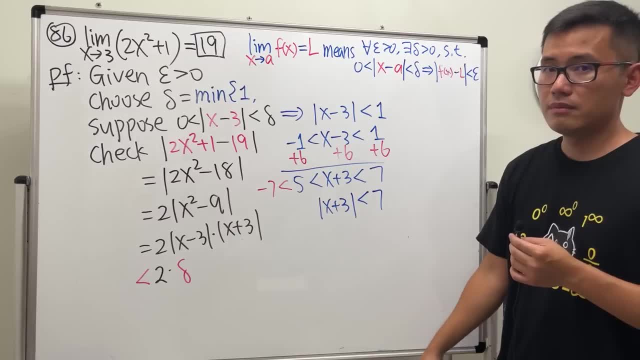 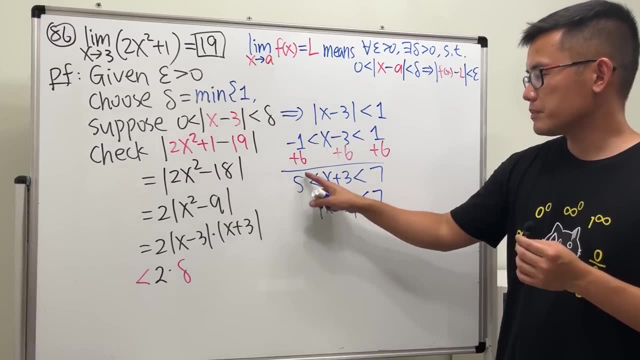 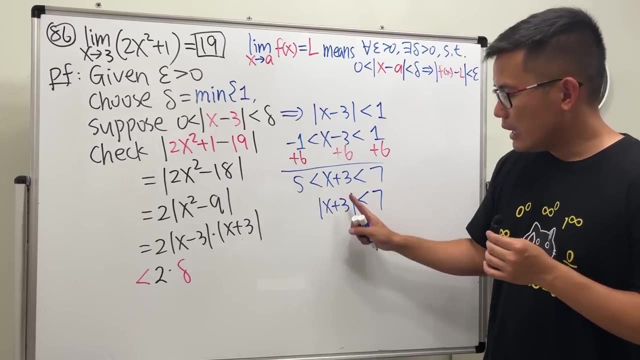 this as absolute value of x, x plus three, less than seven. yeah, and later you're going to see a slightly strange case, but for now just remember, look at which number has a bigger absolute value. so you know what? now you see we have this. absolute value of x plus three is: 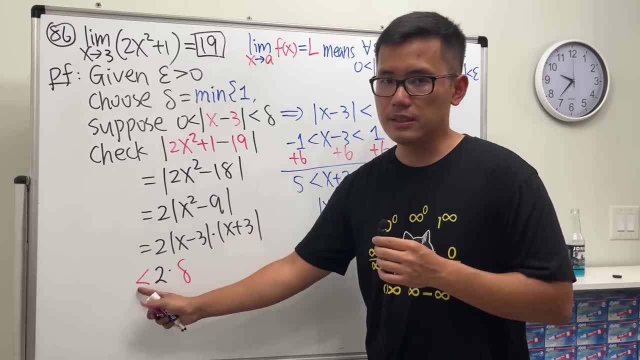 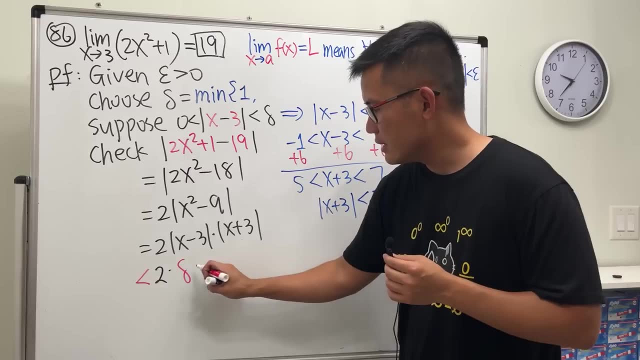 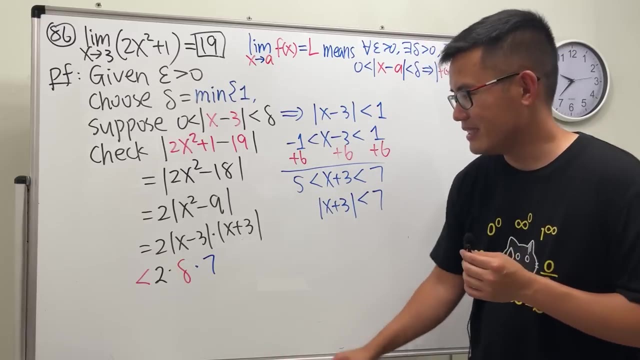 less than seven. this is great, because this is less than we have, less than already. we don't have to write it again. this is not a list. you just say that this right here is less than seven. yeah, yay, seriously, okay. now question: what's your delta? b, though, because again, 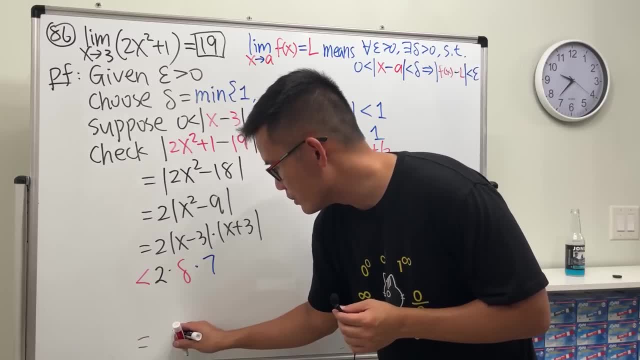 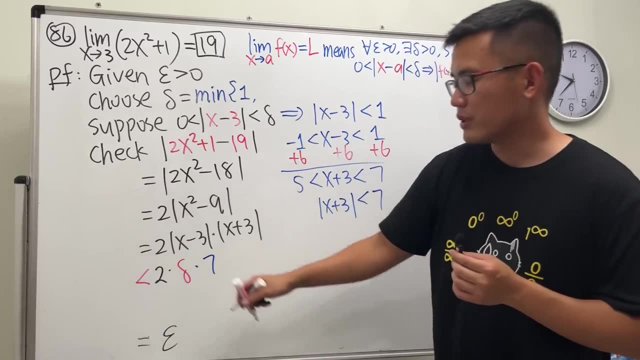 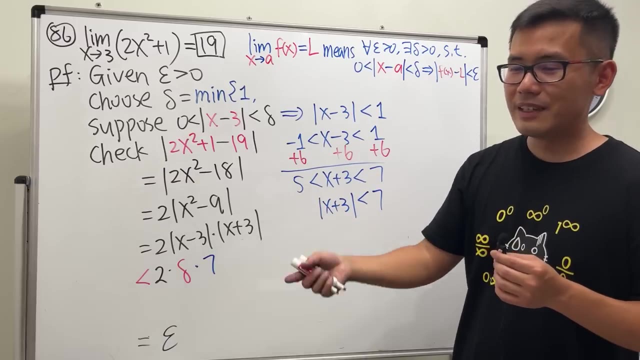 at the very end. we want to have this to be just delta. so we just want to have this as just epsilon. so what should be delta? b? two times seven is, i wanted to say, 17.. two times seven is 14.. so we better have: 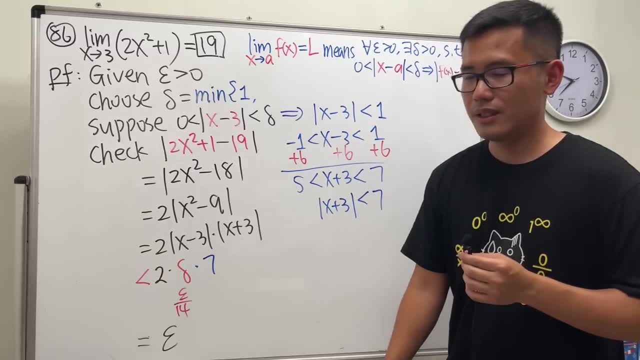 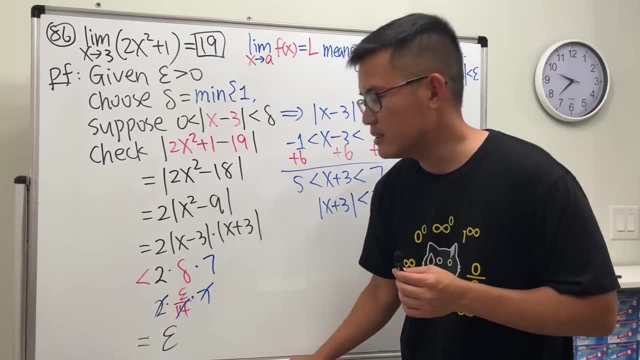 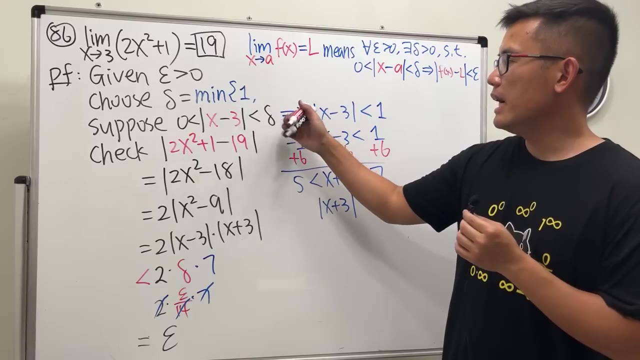 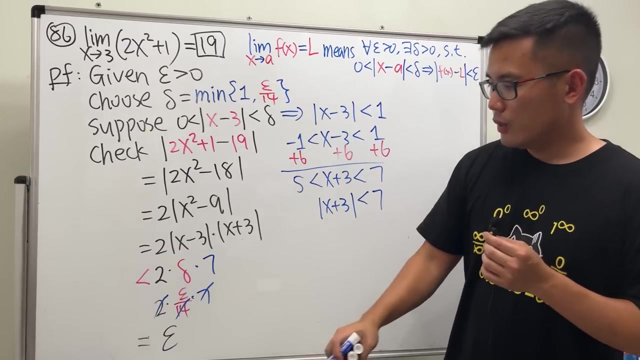 delta to be epsilon over 14, so that you see two times seven this, this, and that will cancel. now delta, we said, is epsilon over 14. we come back here and then we put down epsilon over 14. close this right here, that we do not put on equal sign because we say delta is the minimum. 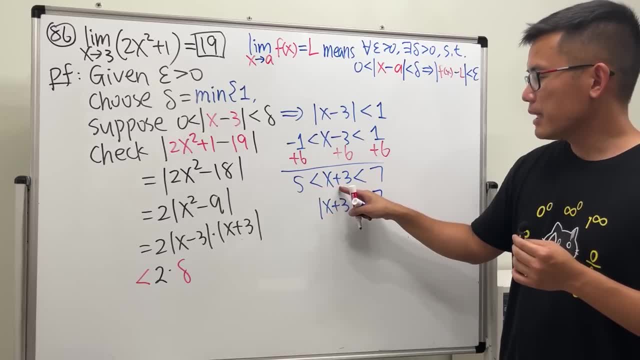 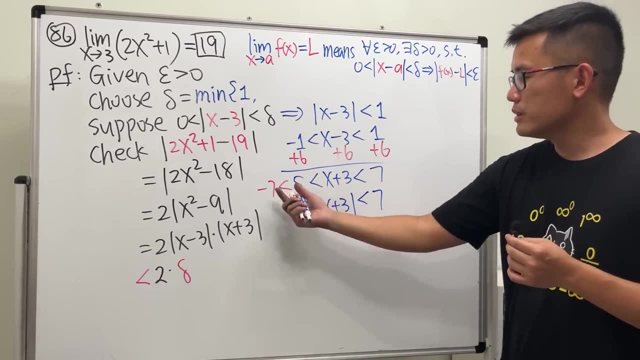 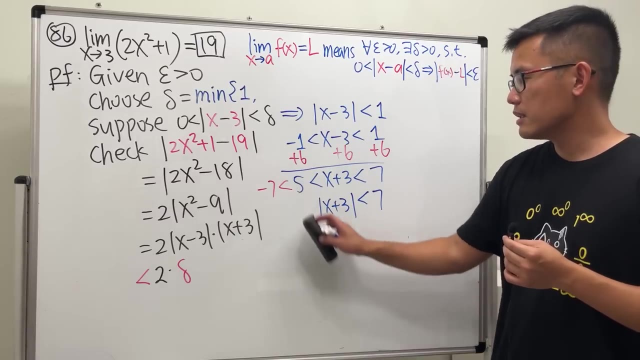 we have this, of course: x plus three. If it's greater than five, it has to be greater than negative seven. so you see that we have negative seven, also seven. so of course we can write this as absolute value of x plus three, less than seven. yeah, and later you're going to see a slightly strange case, but for now just remember. 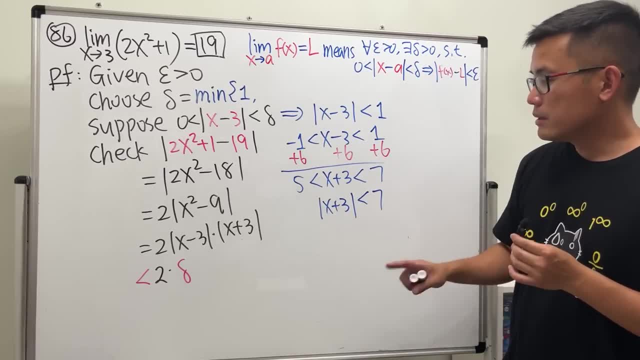 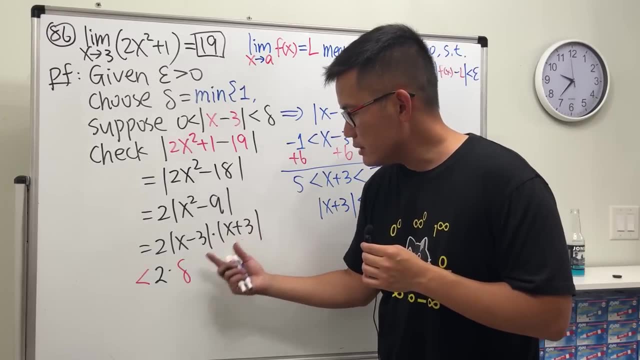 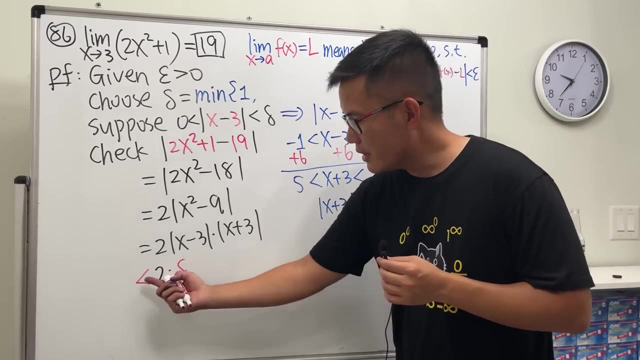 look at which number has a bigger absolute value. so you know what? now you see, we have this absolute value of x plus three is less than seven. this great, because this is less than we have, less than already. we don't have to write you again. this is not a list. you can just say that this right here is less. 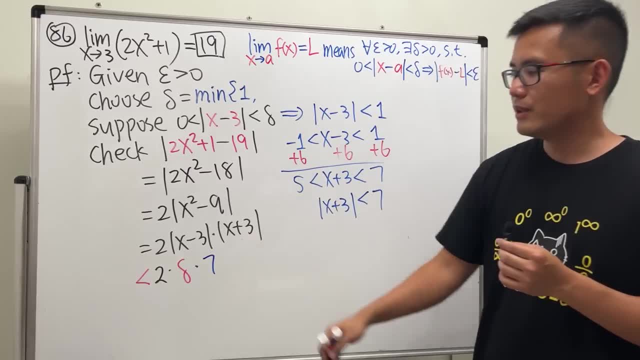 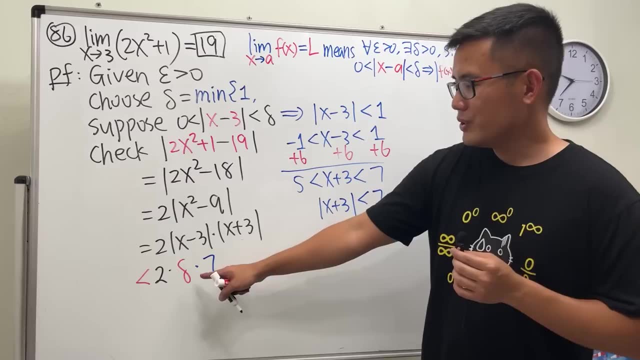 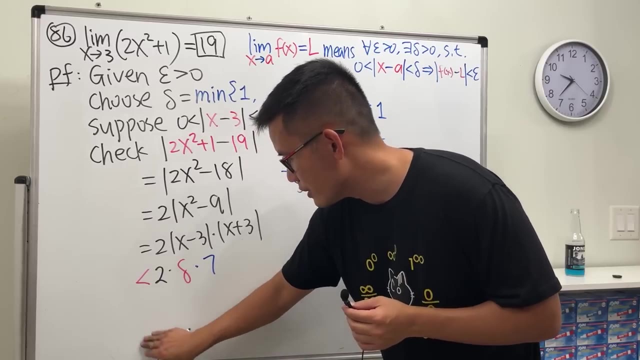 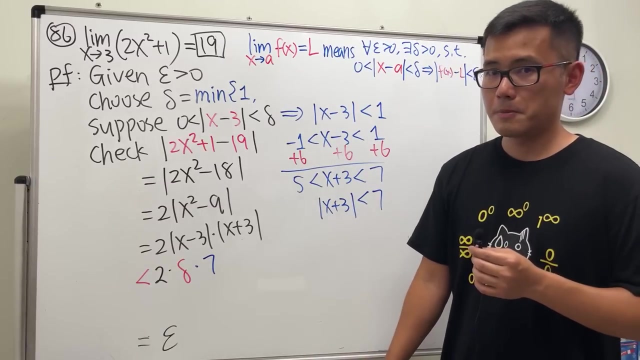 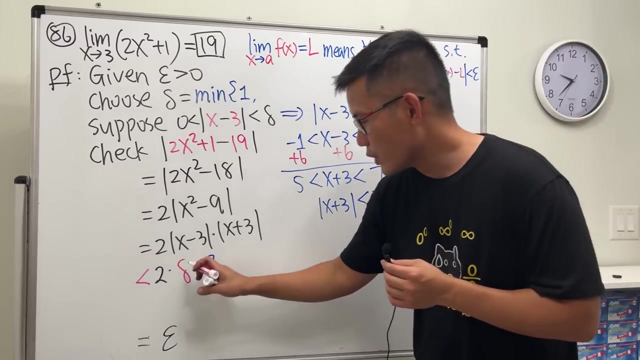 than seven. yay, yay, seriously, okay. now question: what's your Delta V? though? because, again, at the very end, we want to have this to be just Delta, so we would you just want to have this as just epsilon. so what should you copy? 2 times 7- this I wanted to say: 17. 2 times 7 is 14, so we better have Delta to be epsilon. 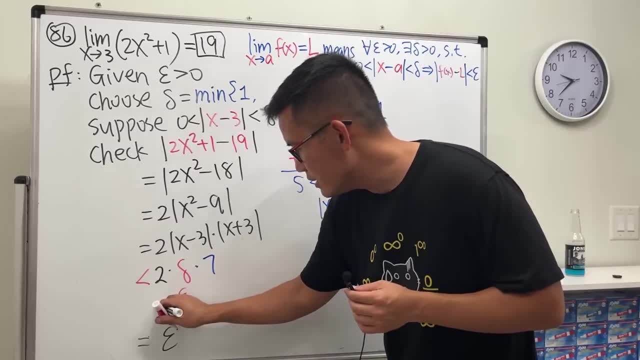 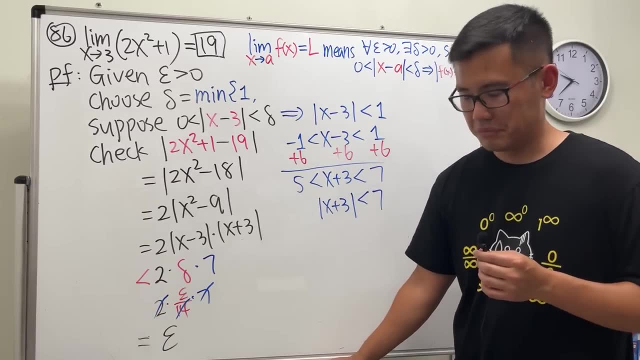 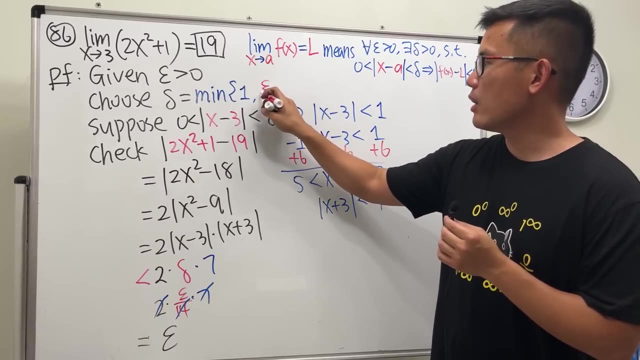 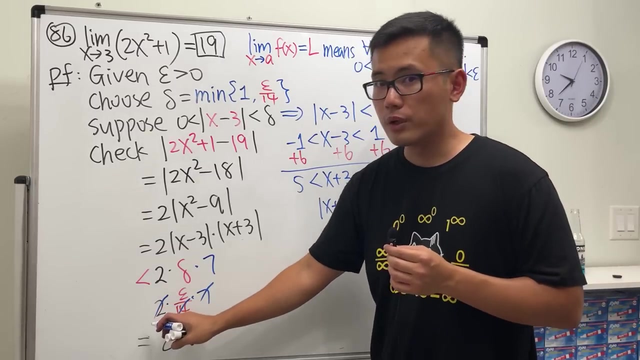 over 14, so that you see 2 times 7 this, this and that will cancel. now Delta, we say this: epsilon over 14. we come back here and then we put down epsilon over 14, close this right here, that we do not put on equal sign because we say Delta is the minimum of 1 or epsilon over 3. so 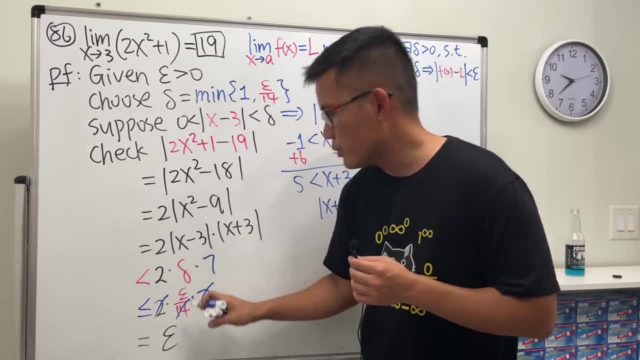 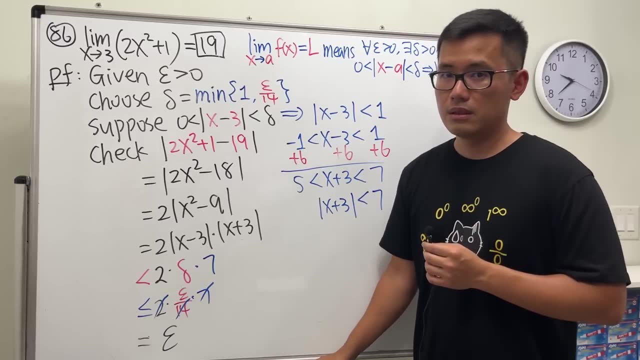 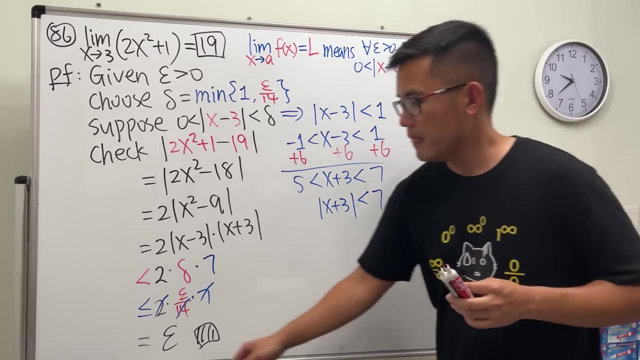 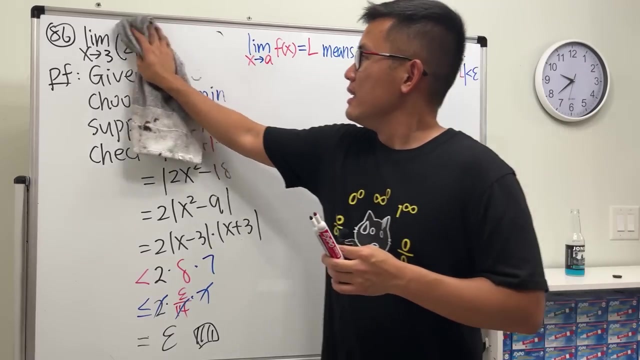 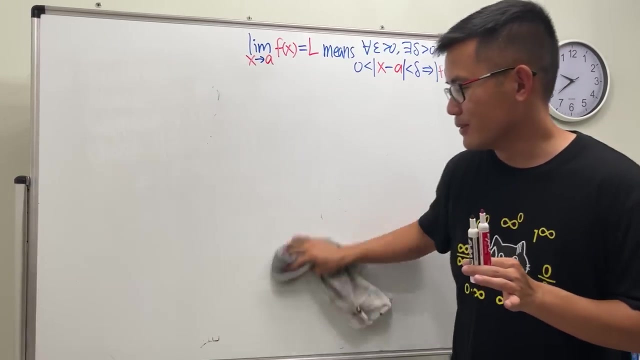 it's a minimum. we want this right here to be less than we equal to. I guess Delta is less than this. what that? okay, well done, well done, right, cool. please do not ask me to do 100 apps on Delta definition, please. no, no, 10 is it's. 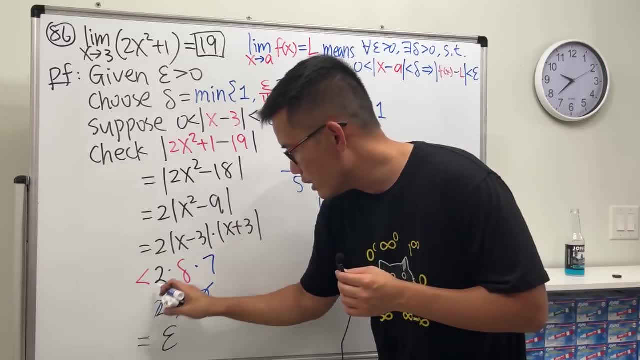 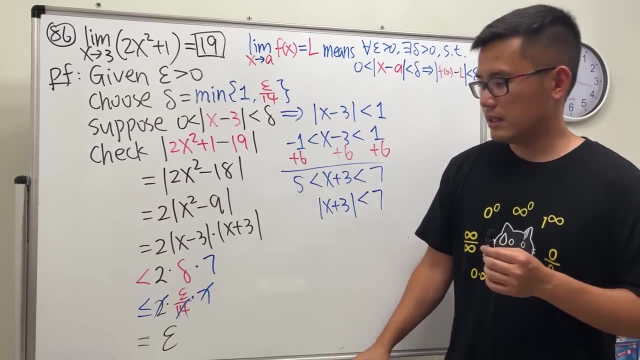 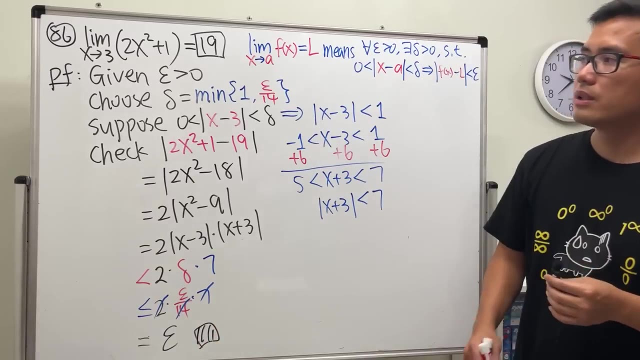 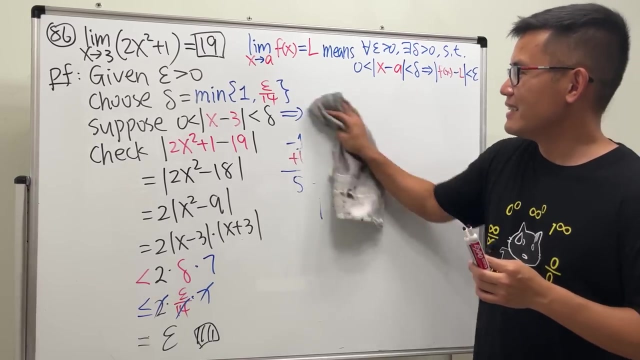 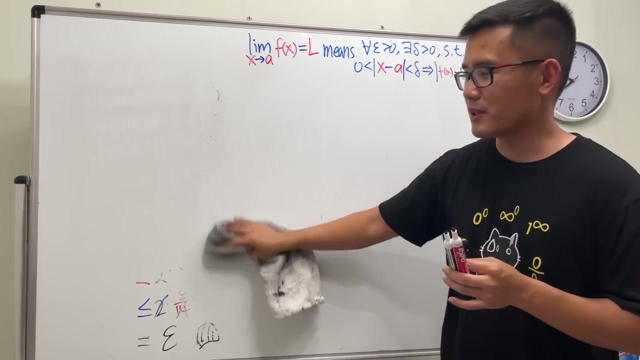 of one or epsilon over three, so it's a minimum. we want this right here to be less than or equal to, because delta is less than this or that. okay, we're done. we're done, we're done. okay, cool, please do not ask me to do 100 apps on delta definition, please. no, no, 10 is it's good. 10 is good. 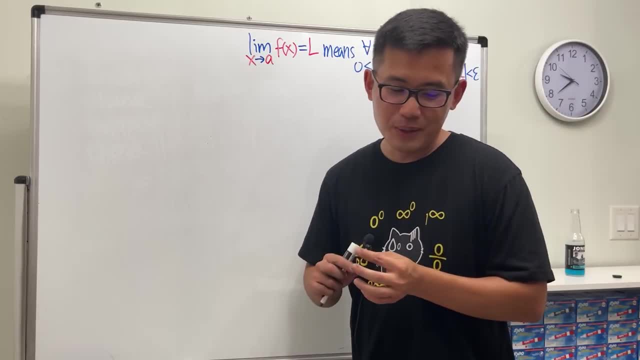 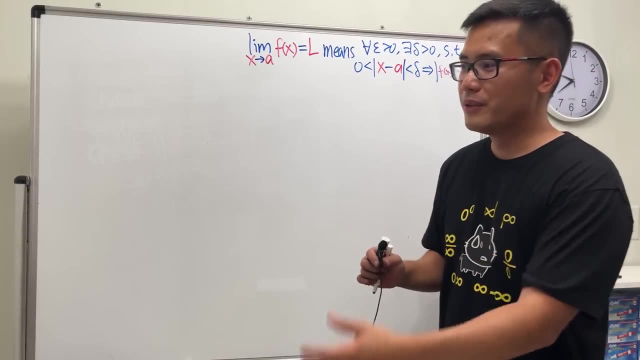 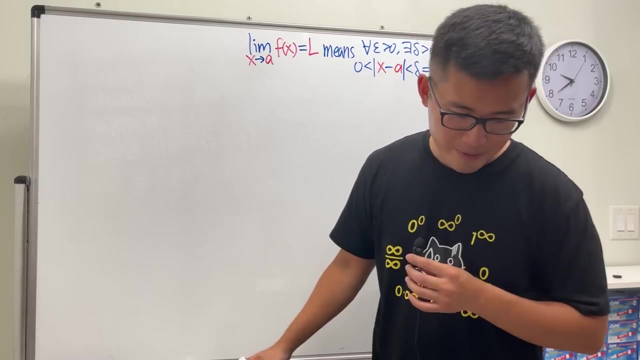 please don't, because this right here are still like to be honest- like an introductory level when we're talking about real analysis. there are crazy stuff, such as proof: a function is uniformly continuous. what dance you have like so many? that's not kid, let's not talk about it, okay. 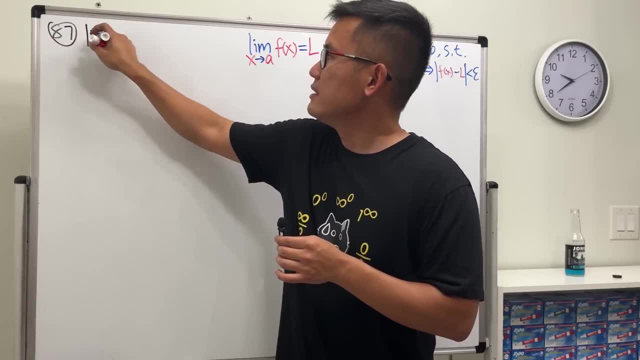 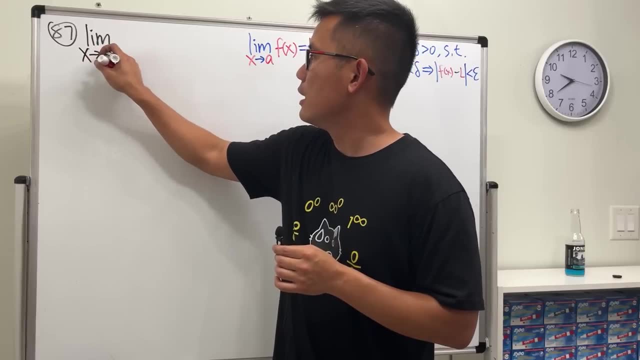 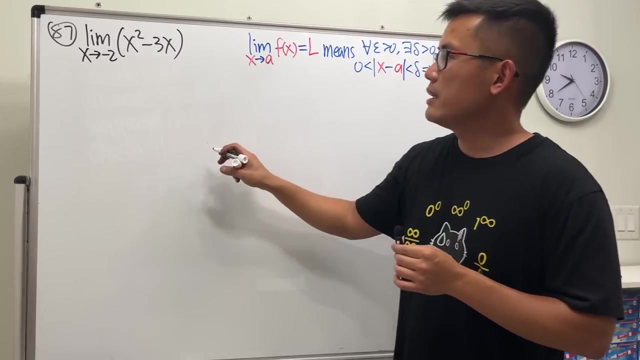 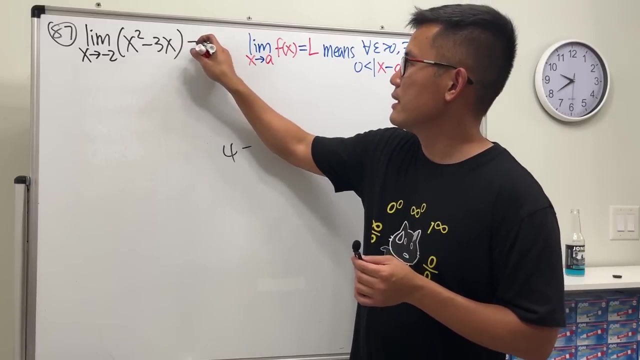 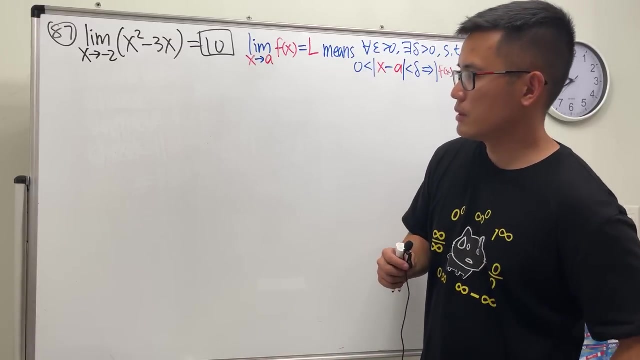 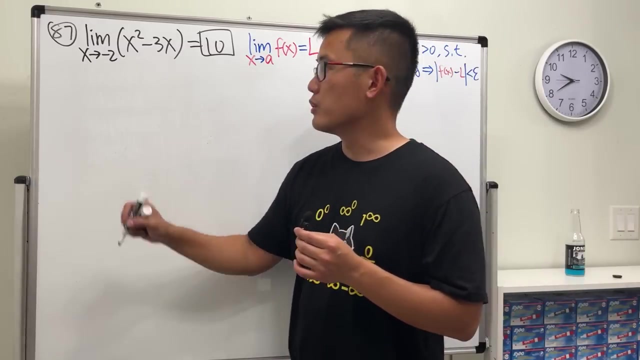 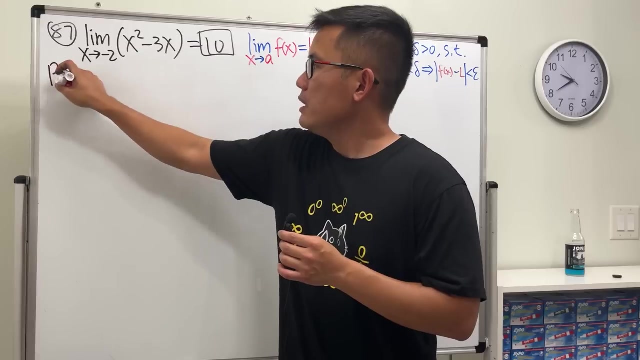 possible, excuse me. okay, 87 limit and we have X approaching negative 2. good, alright, so now again, just go ahead and prove it. this is a quadratic case, so it will be very similar to what we did earlier. so here we go. pf. 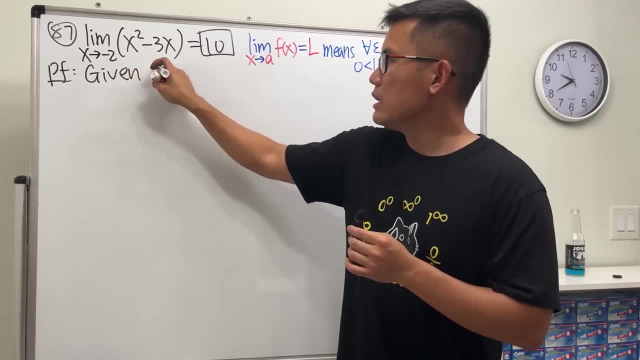 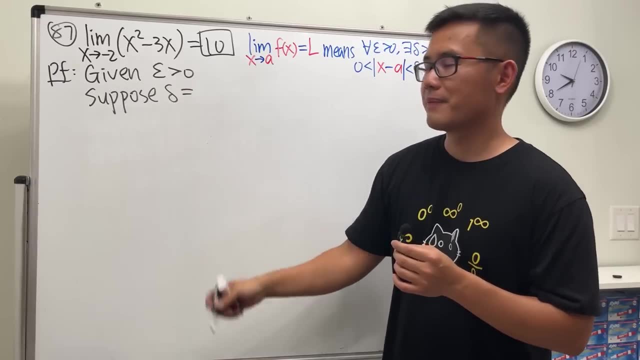 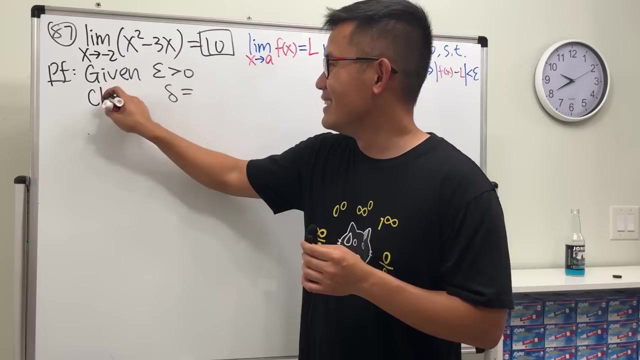 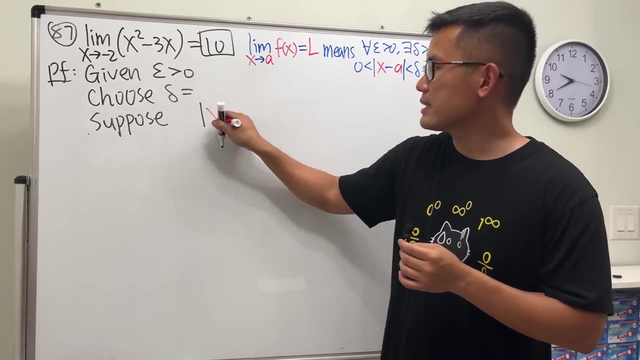 let's go ahead and say: given epsilon greater than 0, and then suppose delta is equal to something, then no, no, no given. choose, sorry, I'm tired choose. suppose, here we go. absolute value of x minus negative 2, so it becomes plus 2. 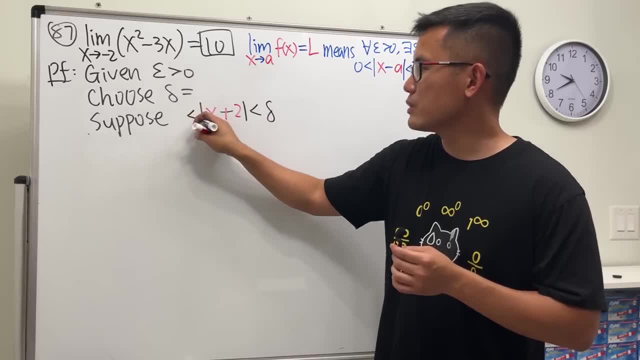 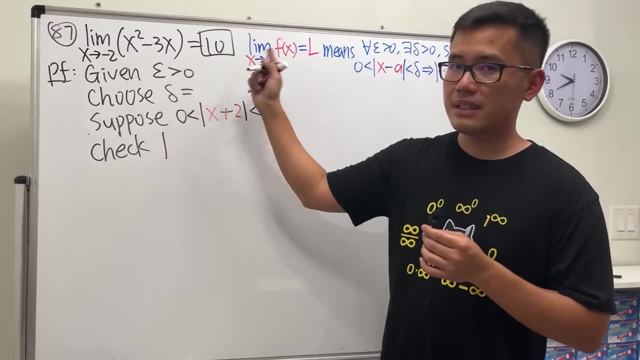 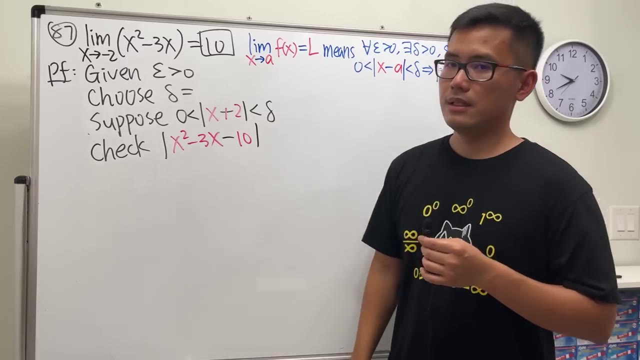 is less than delta, and then this is greater than 0, and then we want to check absolute value function minus the limit. so x squared minus 3x and then minus 10. oh my god, look at this. how beautiful is this. this is a quadratic trinomial. 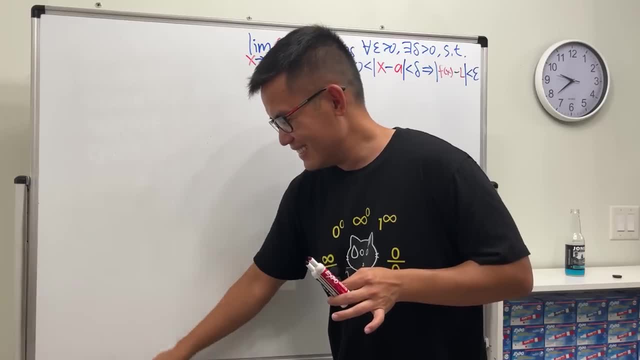 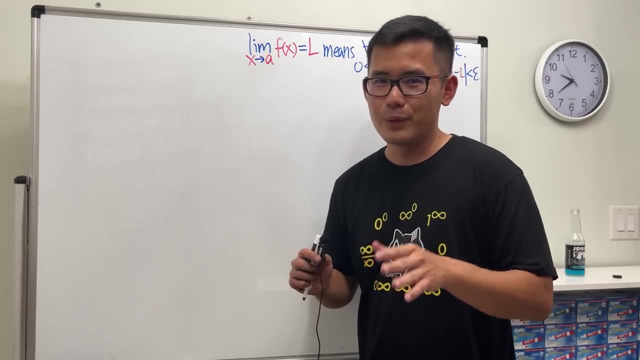 good. 10 is good. please don't because this right here are still like to be honest like an introductory level when we're talking about real analysis. we're still like to be honest like an introductory level when we're talking about real analysis. we're still like to be honest like an introductory level when we're talking about. 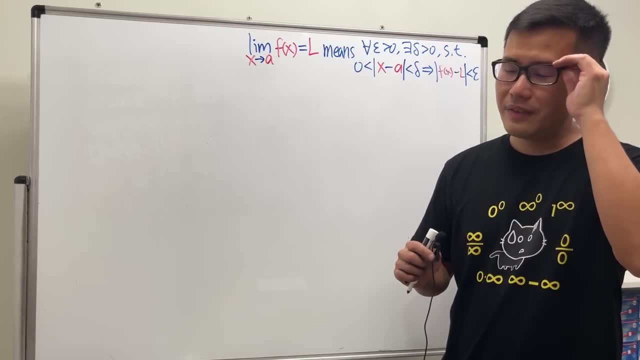 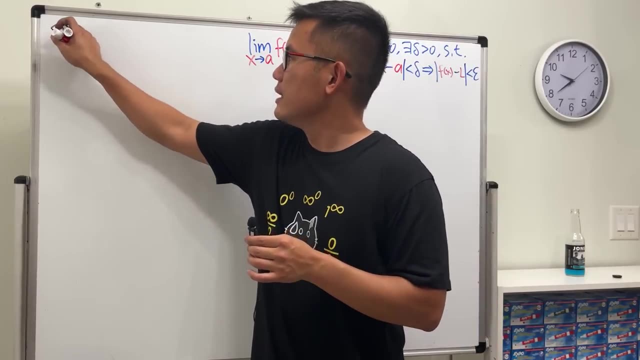 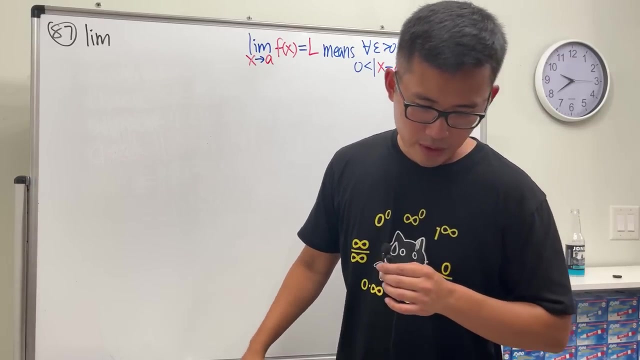 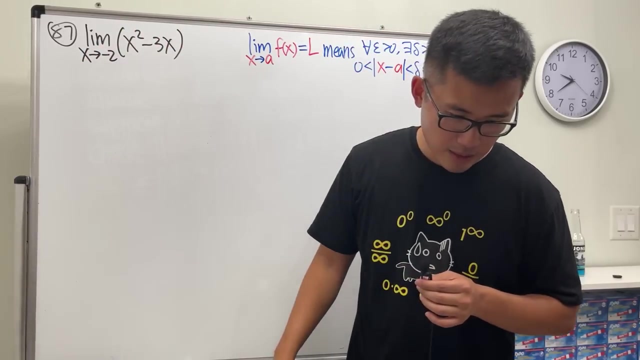 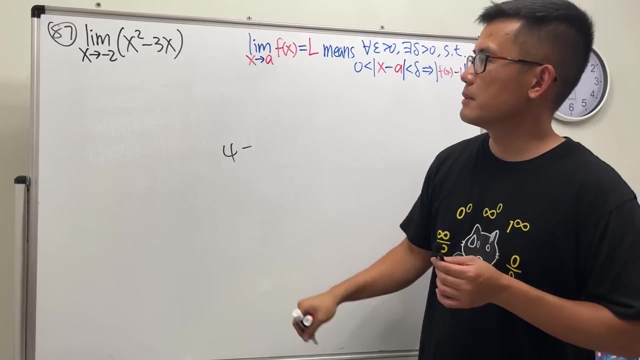 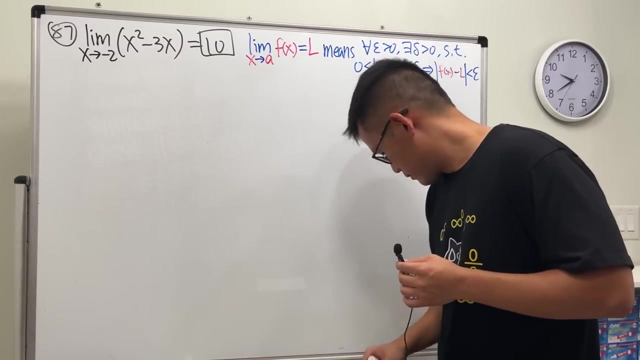 off course for you. if you do ask me, really do ask what is the answer. I don't gonna talk about all the answers. the other days we just going to keep saying weiter 不生死. in here you get four minus three six, so it's ten, right good. 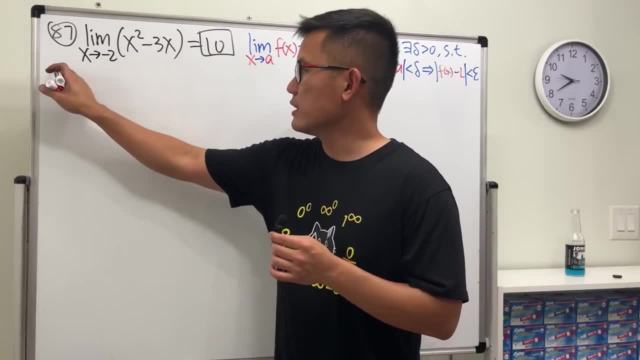 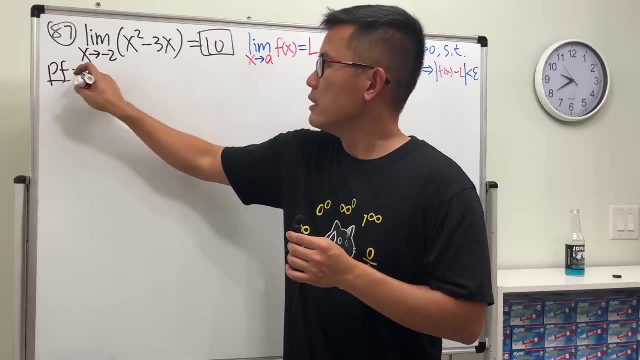 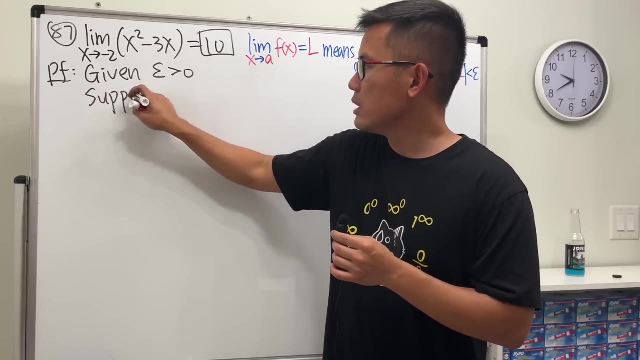 all right. so now again, just go ahead and prove it. this is the quadratic case, so it will be very similar to what we did earlier. so here we go. p, f. let's go ahead and say, given epsilon greater than zero, and then suppose delta is equal to something. then 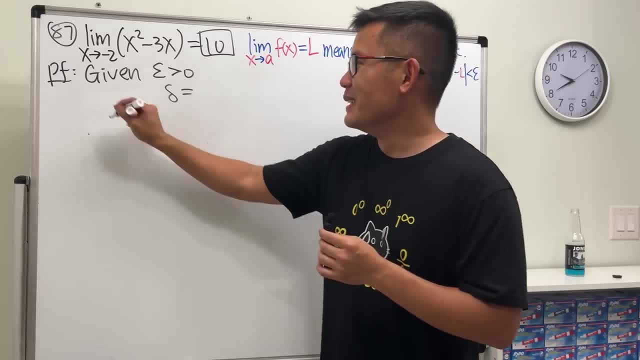 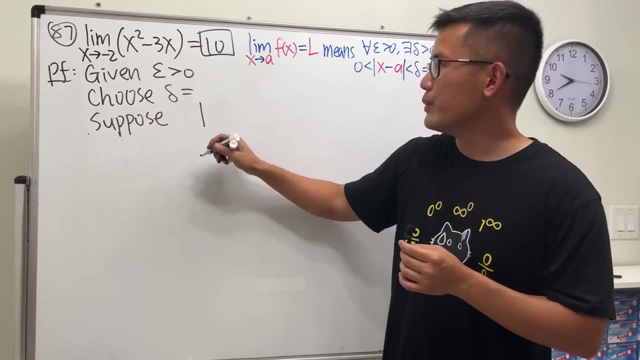 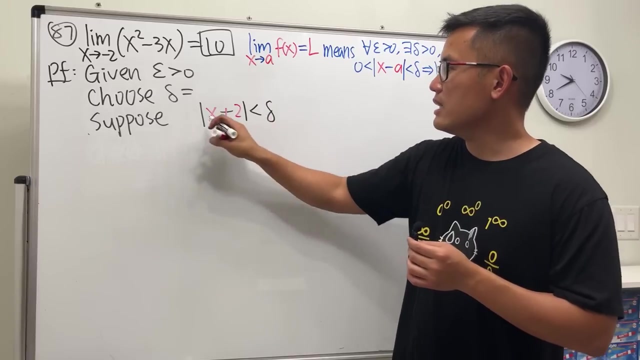 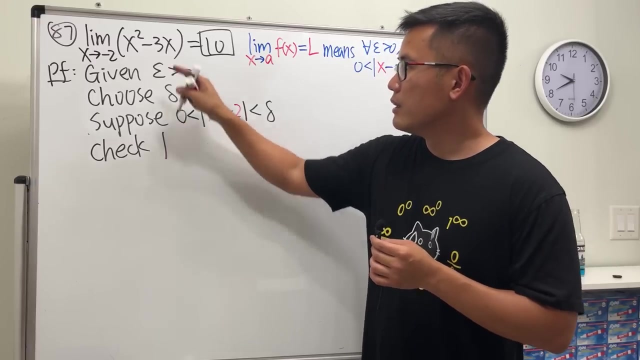 no, no, no, no given. choose, sorry, i'm tired, choose. suppose here we go: absolute value of x minus negative 2, so it becomes plus 2 is less than delta, and then this is greater than zero. and then we want to check absolute value function minus the limit, so x square minus 3x, and then 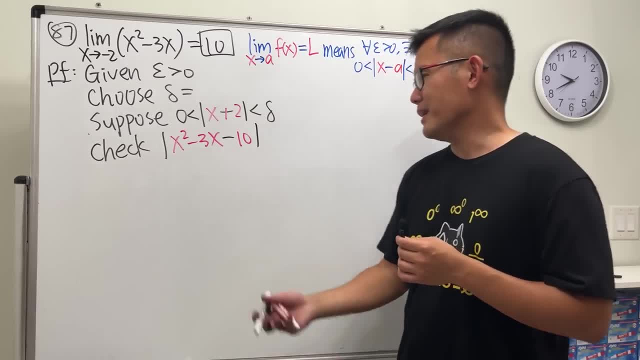 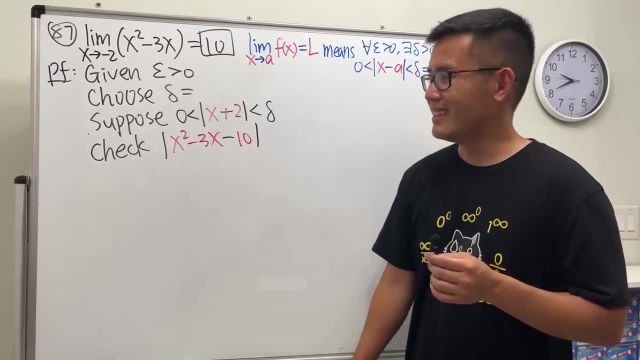 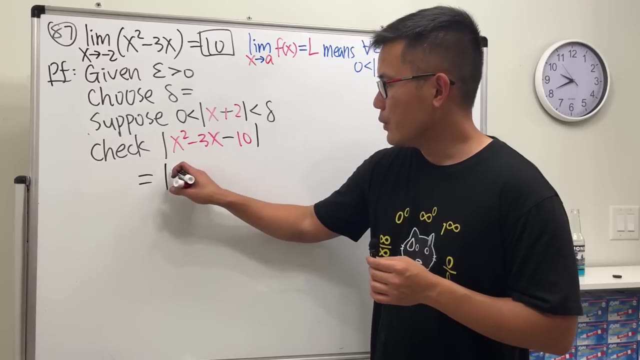 minus 10.. oh my god, look at this. how beautiful is this. this is a quadratic trinomial. we can factor it the usual way. okay, we need x minus 5 times x plus 2. so that's the fact. so here we go: we have absolute value of x. 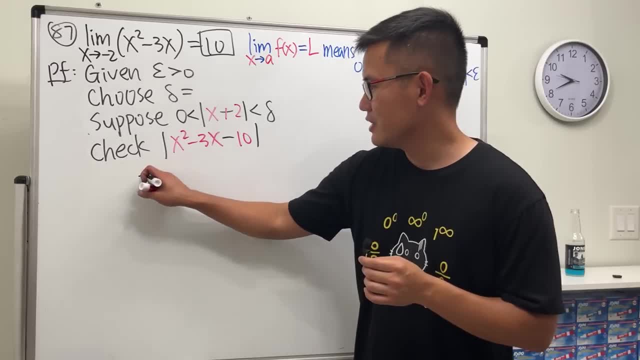 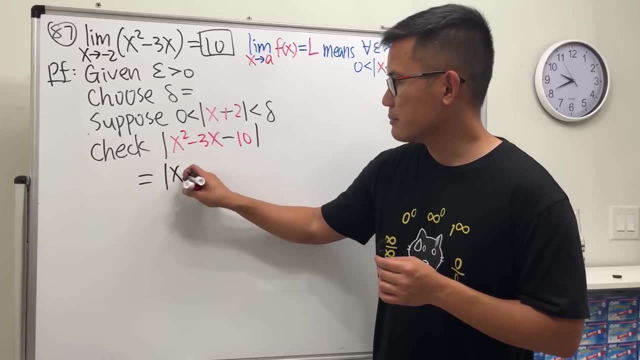 we can factor it the usual way. ok, we need x minus 5 times x plus 2, so that's the factoring. so here we go. we have absolute value of x minus 5. let's put on x plus 2 first, because that way we can put on the delta first. 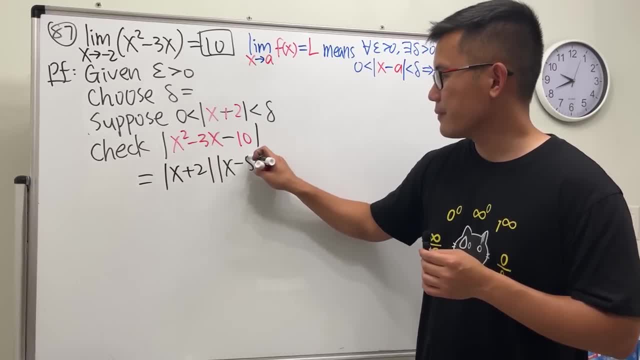 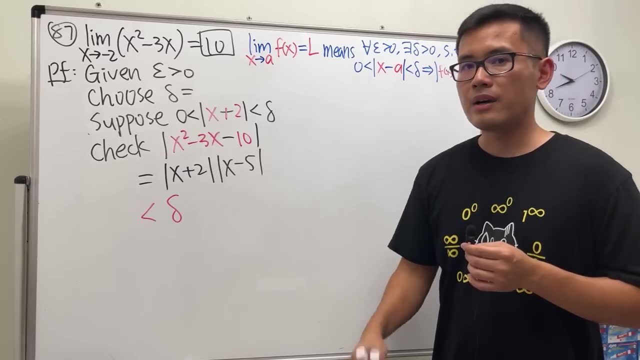 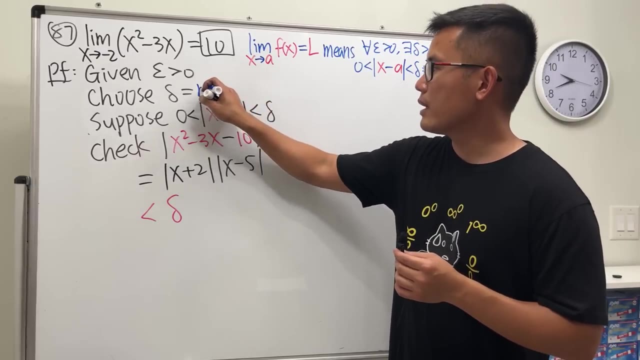 so x plus 2 times x minus 5. ok, this right here is less than delta. that's nice. now we have to get a bound for absolute value of x minus 5. you know the deal. come here and write down minimal. put on 1, just use 1, please. 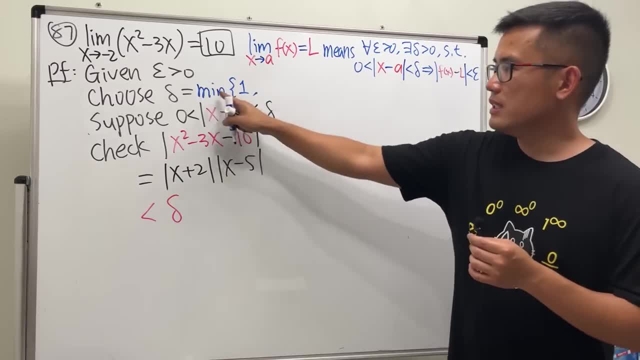 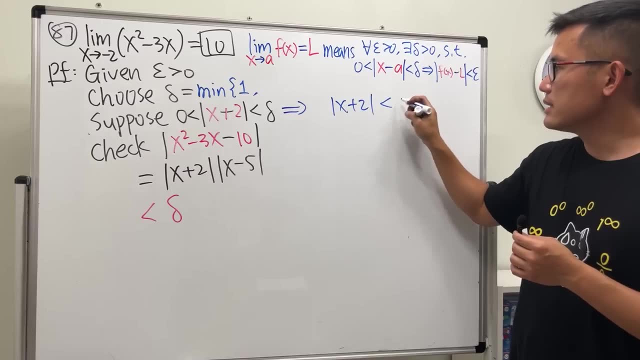 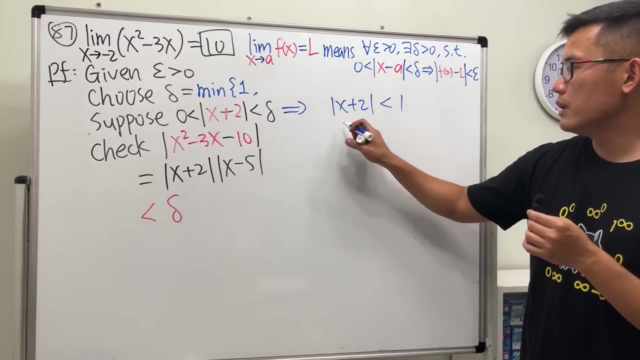 alright, come here. just this side, just this part, so we can say this right here: gives us absolute value of x plus 2 is less than 1, and we want to somehow go from here to here, so let's open. the absolute value that means x plus 2 is in between of: 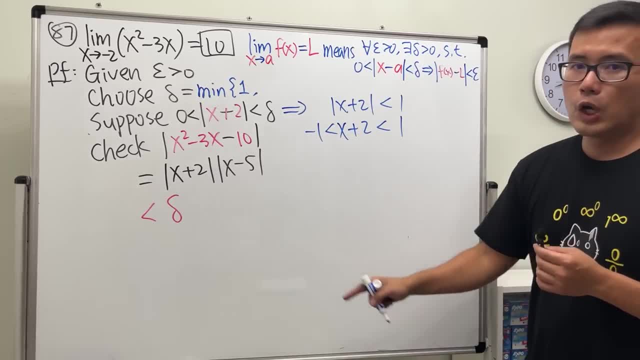 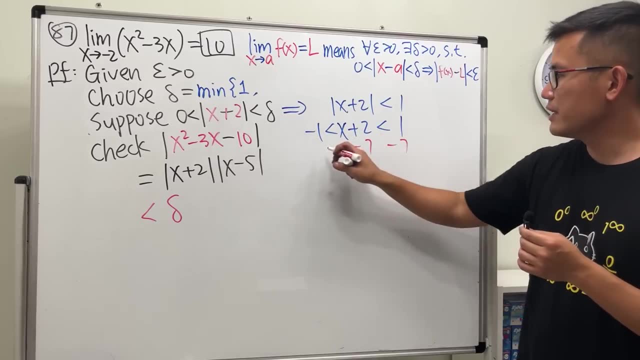 negative 1 and 1. we want to get to negative 5. so that's minus 7 minus 7 here. minus 7 here, minus 7 here, right. so in the middle we have x minus 5. this right here is negative 8. 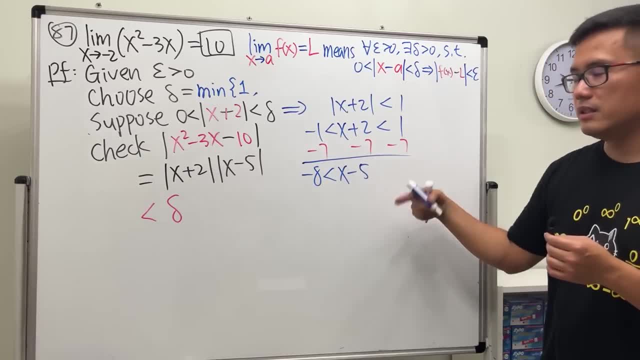 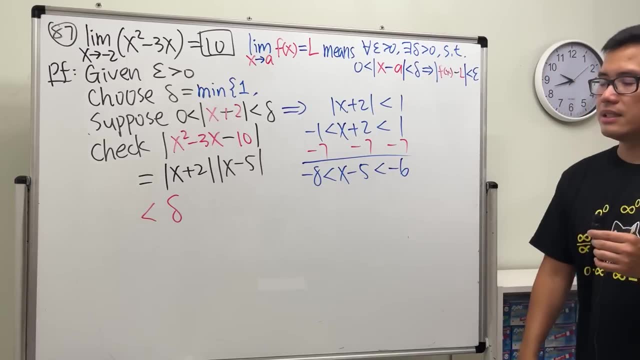 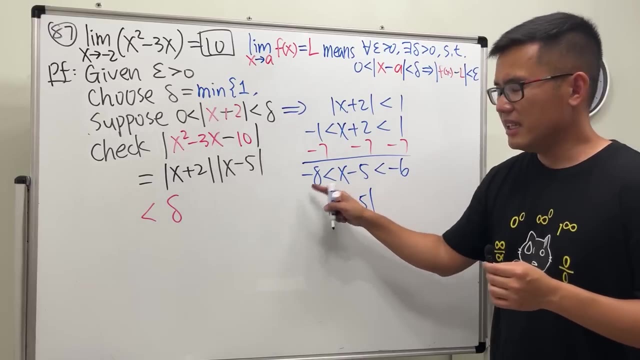 and then I'm just subtracting, so the inequality is maintaining the same. and then less than 1 minus 7 is negative 6. hey, this is crazy, because if we have the absolute value of x minus 5, this is negative, that's negative. I cannot say this is less than negative 6. 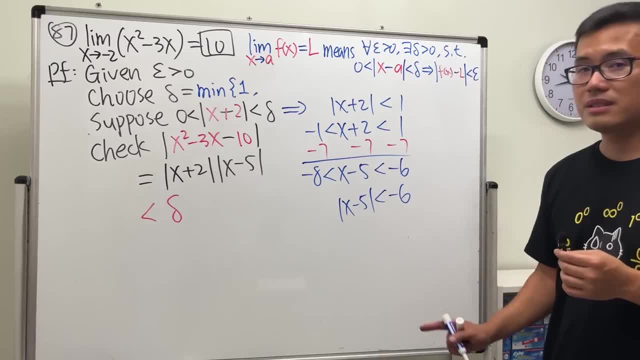 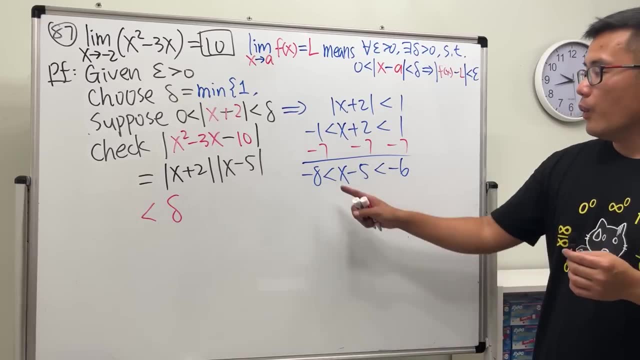 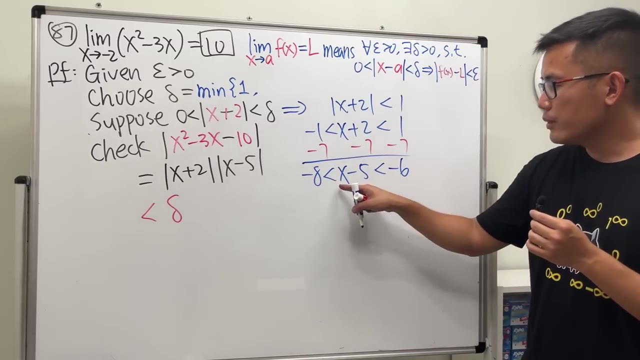 that doesn't make sense. this doesn't make sense. but the deal is that remember what I told you guys earlier: we are looking at which number has a bigger absolute value. I'm not talking about which number is bigger. so I'm telling you guys that, hey, just do absolute value of x minus 5. 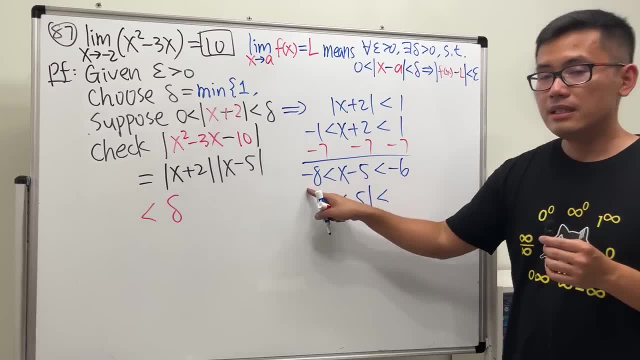 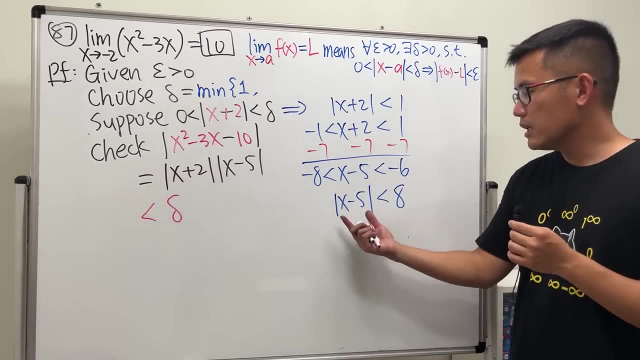 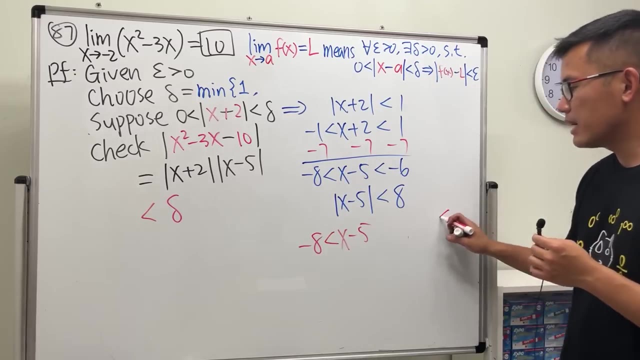 put that as less than the absolute value of negative 8, which is just an 8. why is this true? because here, if you open this, we get what x minus 5 is in between of negative 8 and positive 8. negative 6 is right here. 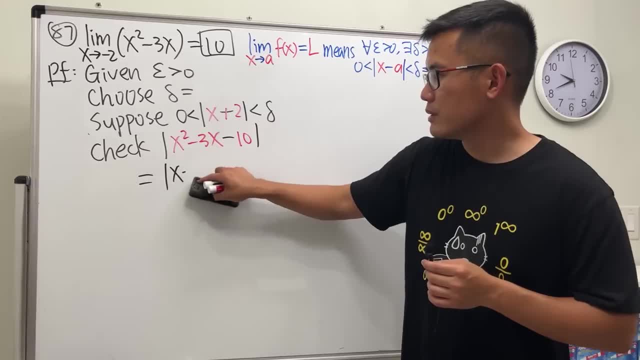 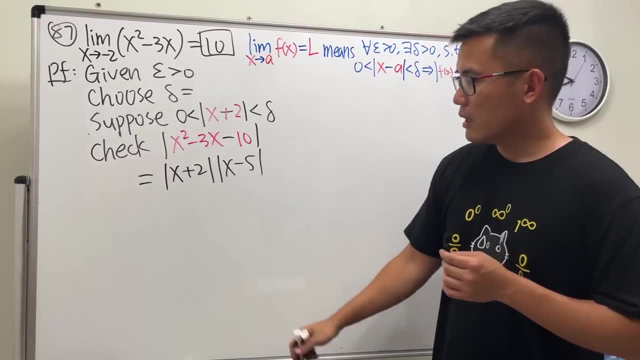 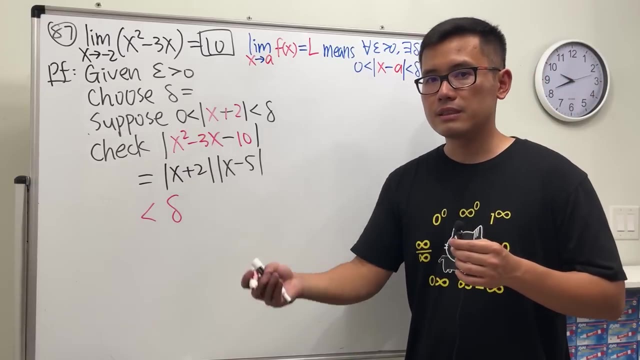 minus 5.. let's, let's put on x plus 2 first, because that way we can put on the delta first. so x plus 2 times x minus 5.. okay, this right here is less than delta. that's nice. now we have to get a bound for absolute value of x minus 5.. you know the deal. come here and write it. 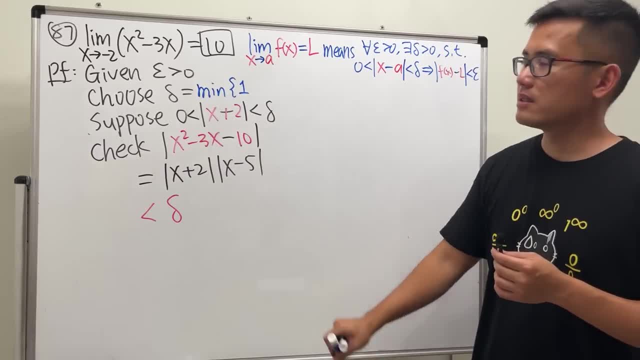 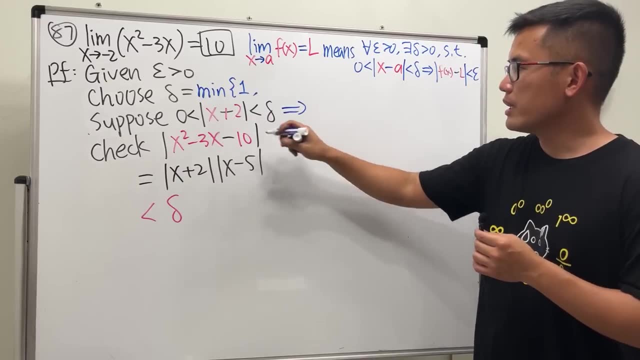 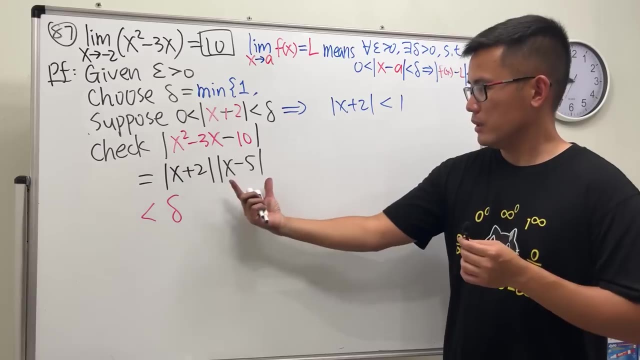 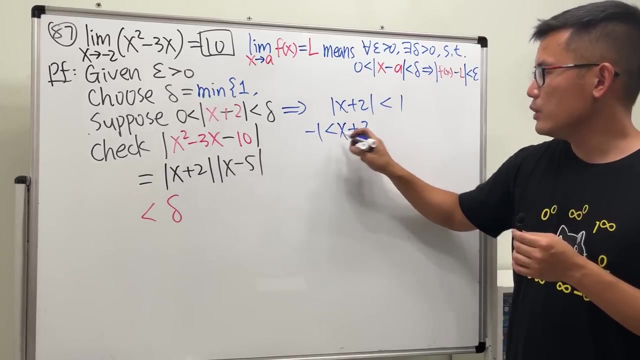 minimum, put on 1, just use 1, please. all right, come here. just this side, just this part, so we can say this right here, gives us absolute value of x plus 2 is less than 1 and we want to somehow go from here to here, so let's open the absolute value. that means x plus 2 is in between of negative 1 and 1.. 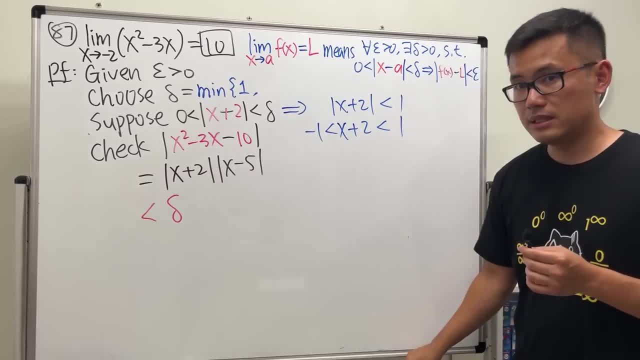 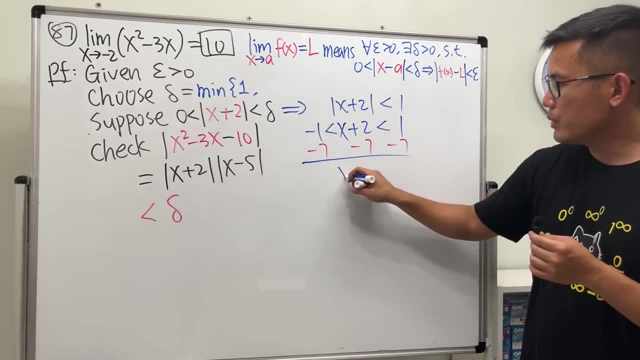 we want to get to negative 5. so let's minus 7 minus 7 here, minus 7 here, minus 7 here, right. so in the middle we have x minus 5. this right here is negative 8. and then i'm just subtracting, so the inequality is: 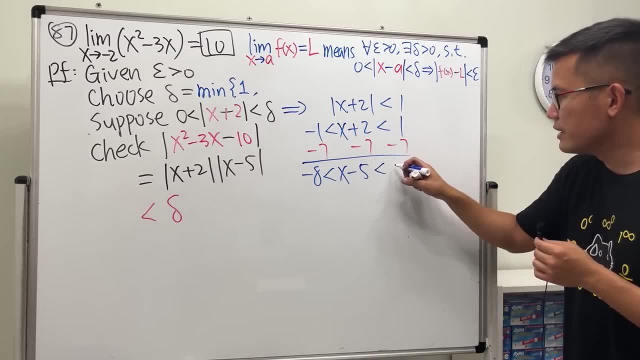 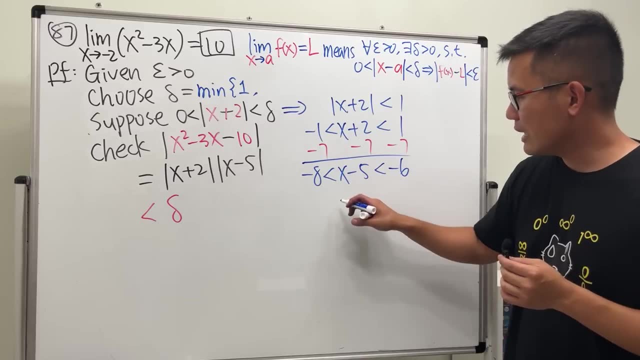 maintaining the same and then less than 1 minus 7 is negative 6.. hey, this is crazy, because if we have the absolute value of x minus 5, this is negative. that's negative. i cannot say this is less than negative 6. that doesn't make sense. 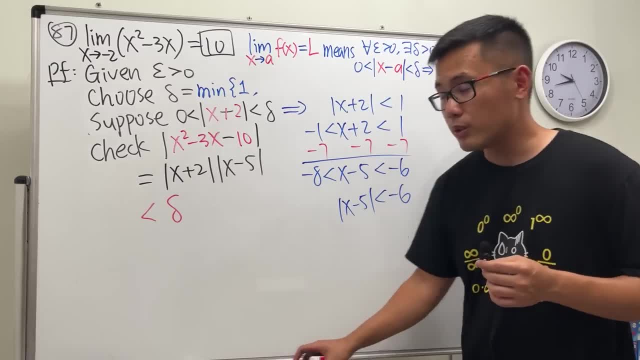 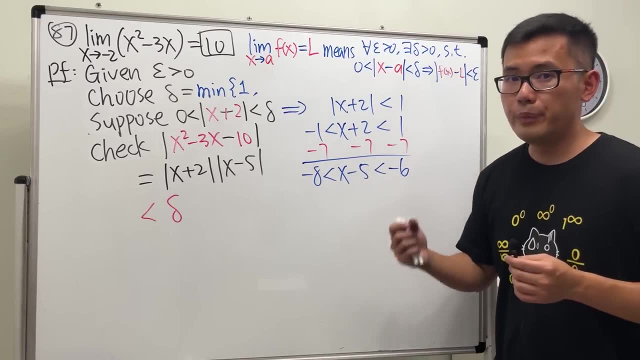 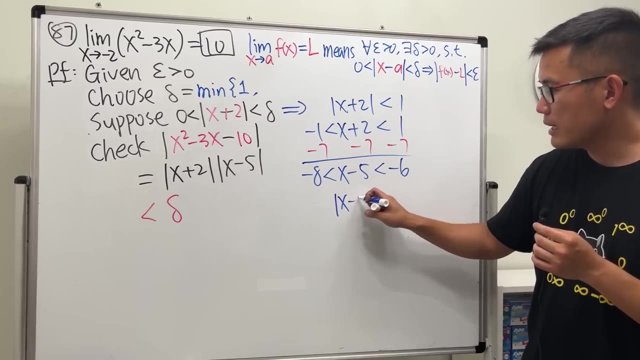 this doesn't make sense, but the deal is that remember what i told you guys earlier: we are looking at which number has a bigger absolute value. i'm not talking about which number is bigger. so i'm telling you guys that, hey, just do absolute value of x minus 5. 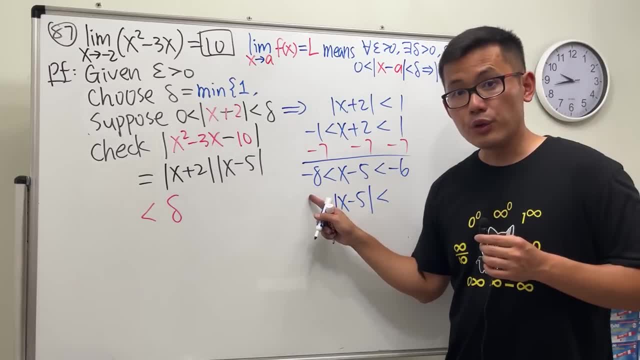 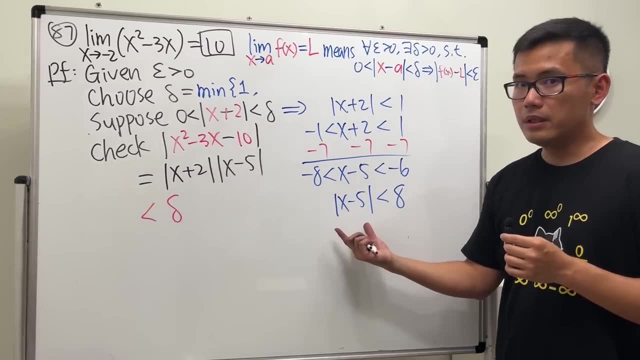 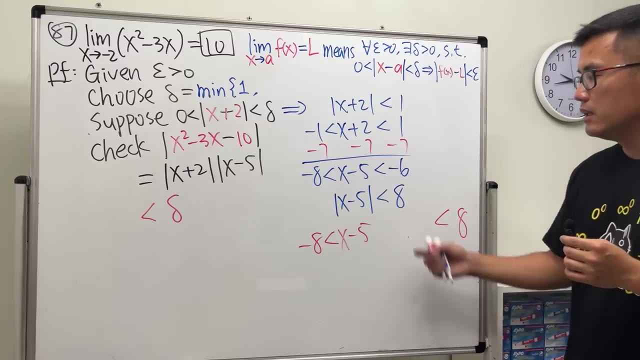 put that as less than the absolute value of negative 8, which is just an 8. why is this true? because here, if you open this, we get what x minus 5 is in between of negative 8 and positive 8.. negative 6 is right here, of course. this covers that situation, all right. 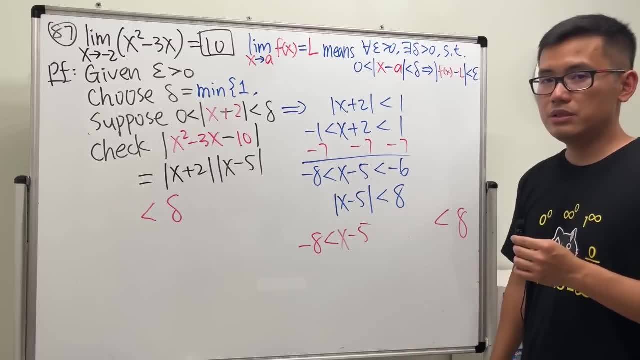 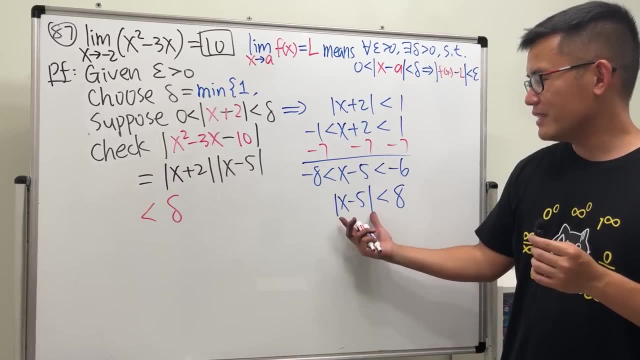 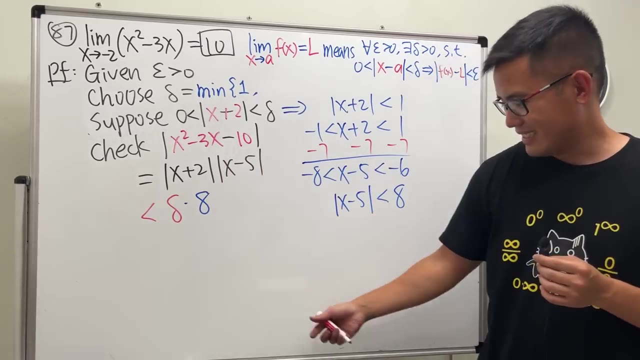 of course this covers that situation, alright. so here we have it. this blue part is this. we can just say, hey, multiply that by 8. that's my delta, that's my 8. at the end, we want to end out with epsilon. so delta should be equal to what? 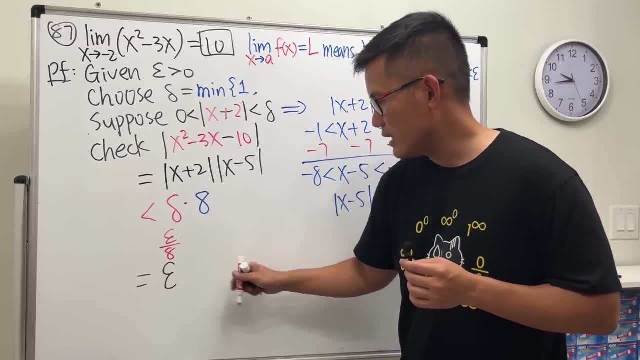 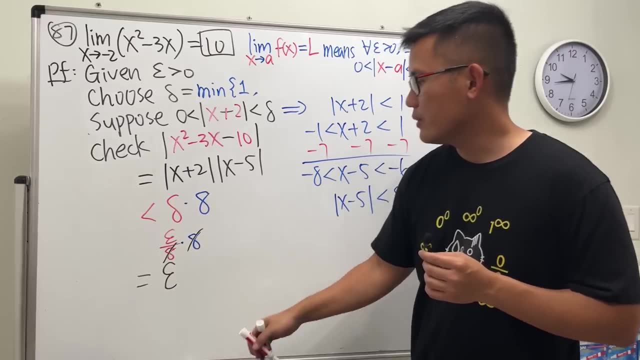 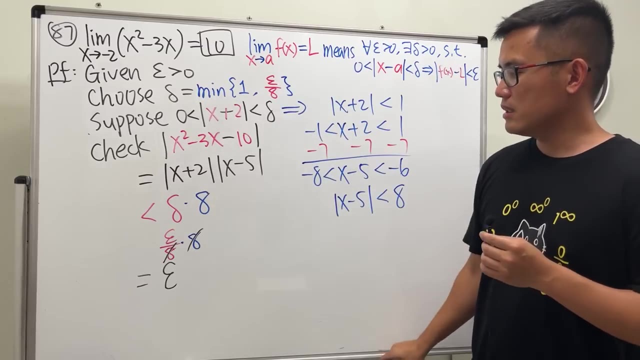 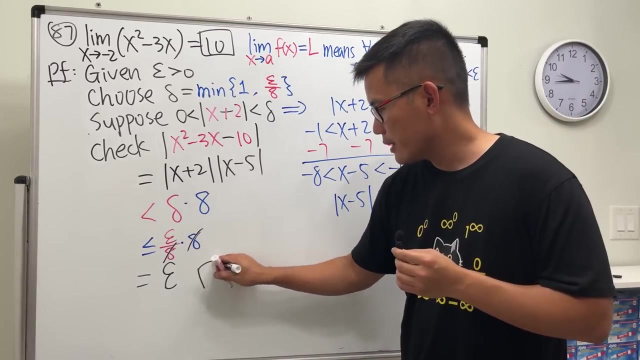 epsilon over 8, yes, let me just write it down nicer for you guys: times 8, cancel, cancel, epsilon over 8, close. that make it legitimate. and then, right here, less than or equal to, because we used the minimum. so this is how you write the proof for it. 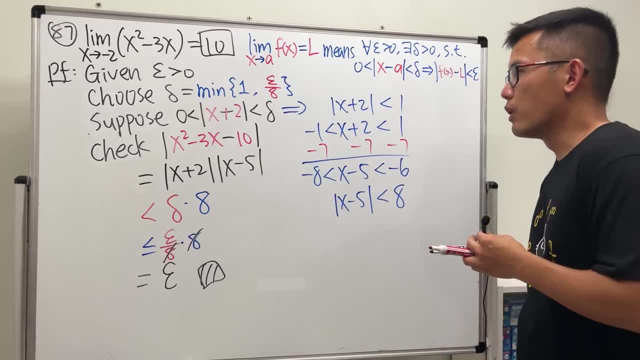 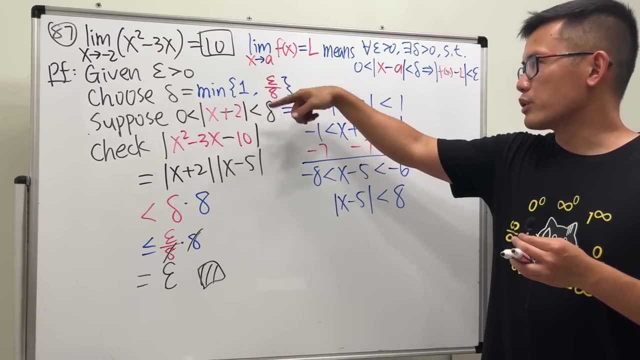 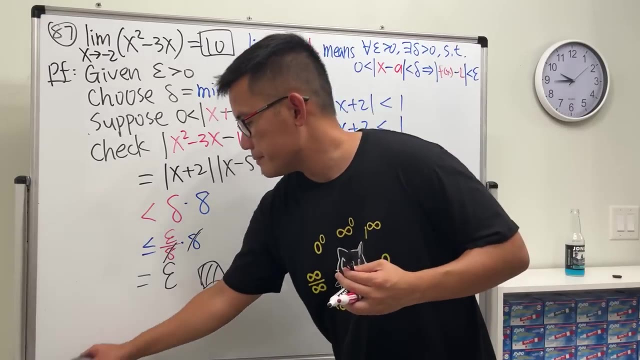 yeah, could there be another choice for delta? yes, because if you use that, say 2, then this delta, this expression, will be different and it will still work theoretically speaking. yeah, but to really understand what's going on for epsilon delta definition, I will highly recommend you guys to watch my video. 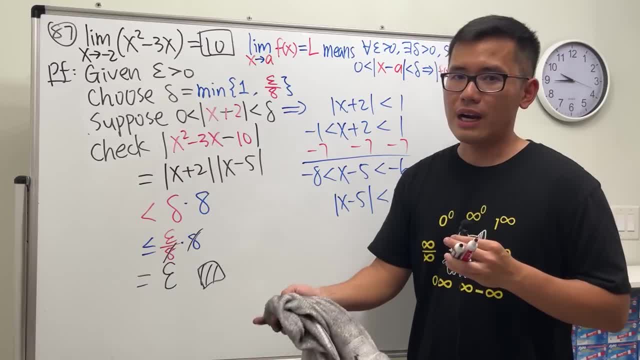 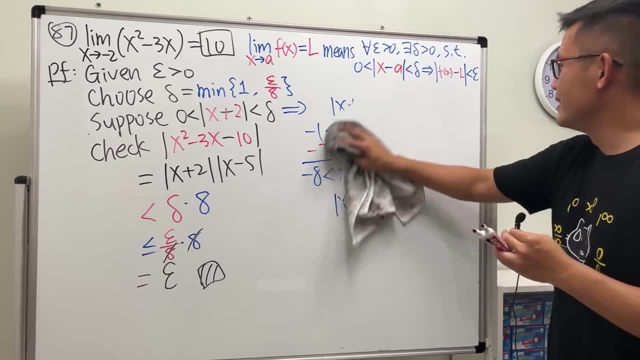 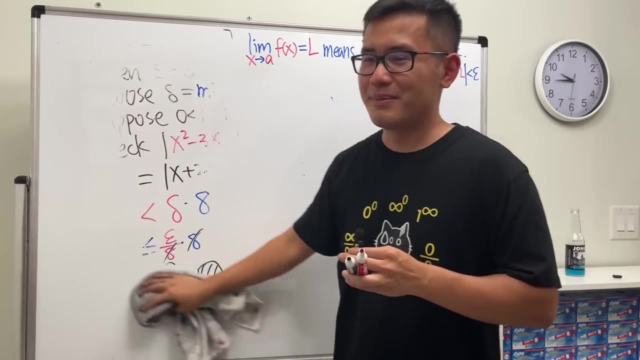 because I use actual example, my actual numbers and also the graph, and I explained it when I'm like when I was like 100% energy- right now, I don't know- I use 78% of my life already, so I have like 13% more. 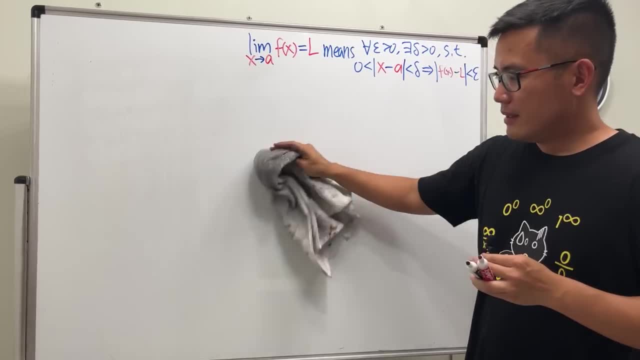 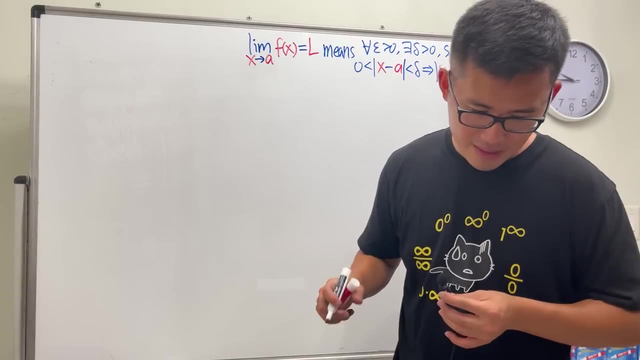 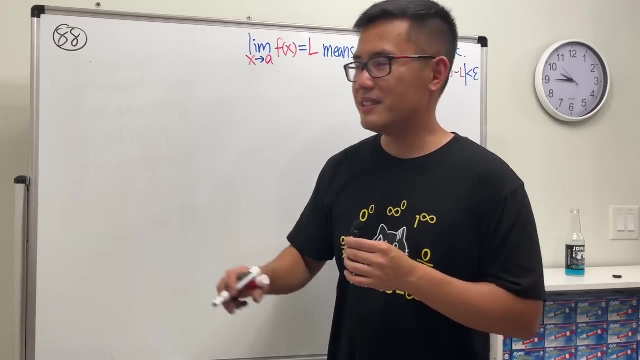 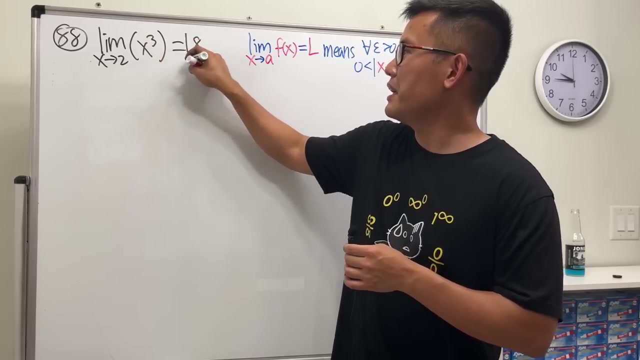 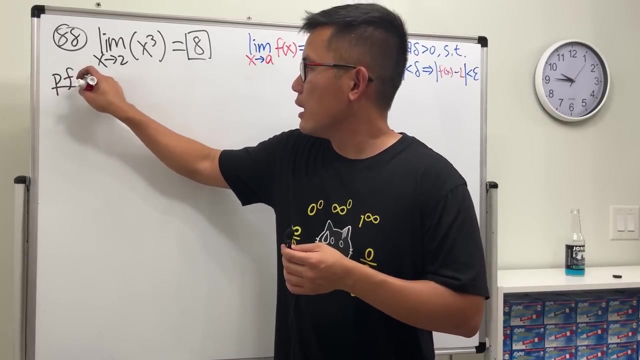 ok, ok, alright now. cubic example. I also picked this one on purpose, number 88. what's the limit as x approaching 2 of x to the third power? you know it's 8, why? ok, this is like extension of the quadratic case, if you have. 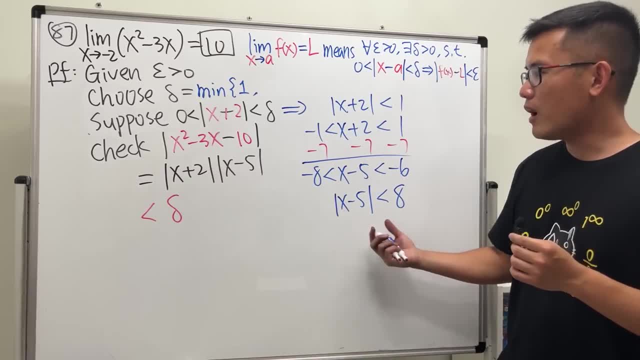 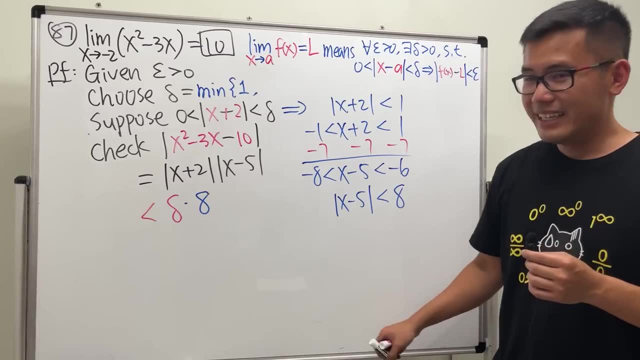 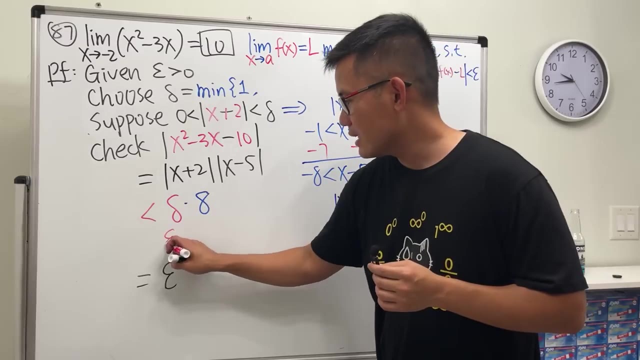 so here we have it. this blue part is this: we can just say, hey, multiply that by 8. that's my delta, that's my 8.. at the end we want to end up with epsilon. so delta should be equal to what epsilon over 8? yes, let me just write it down nicer for you guys: times eight. 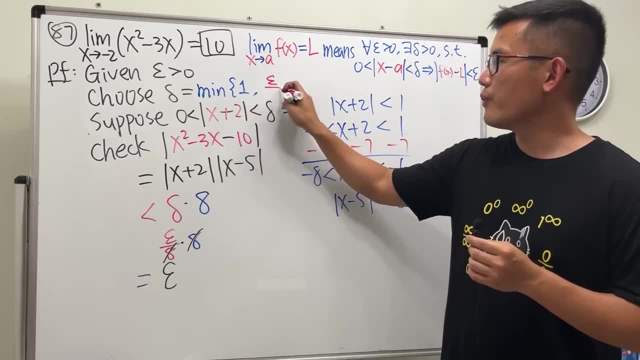 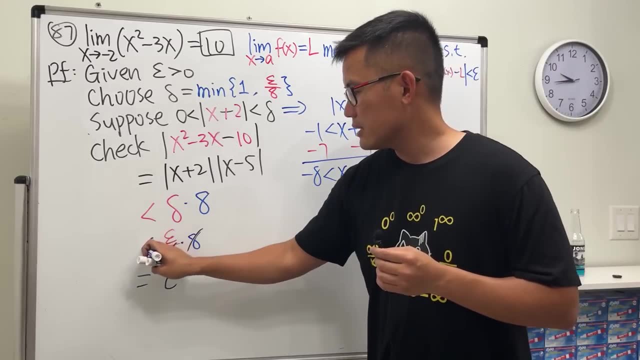 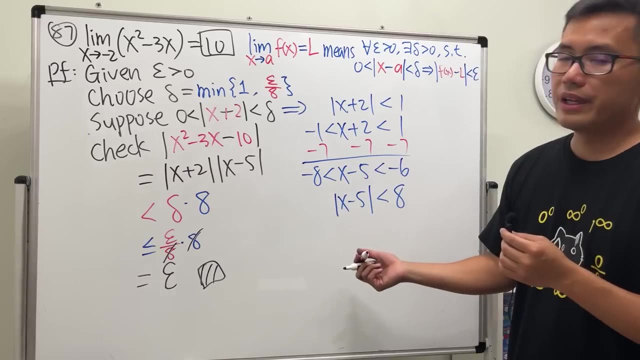 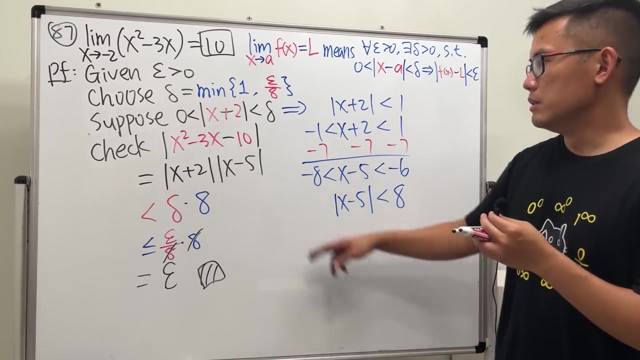 cancel, cancel. come back here: epsilon: over eight, close, that make it legitimate. and then, right here, less than or equal to, because we used the minimum. so this is how you write the proof for it: yeah, could there be another choice for delta? yes, because if you use that, say two, then uh, this delta, this expression will be different. 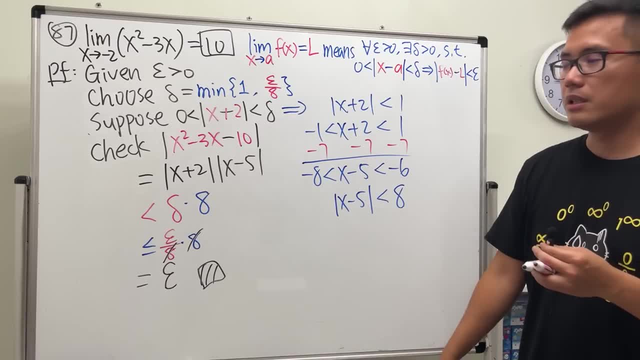 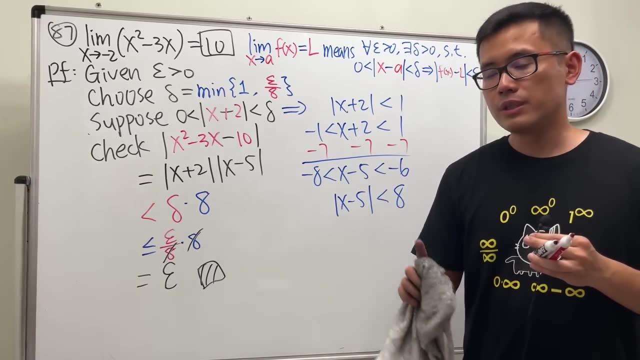 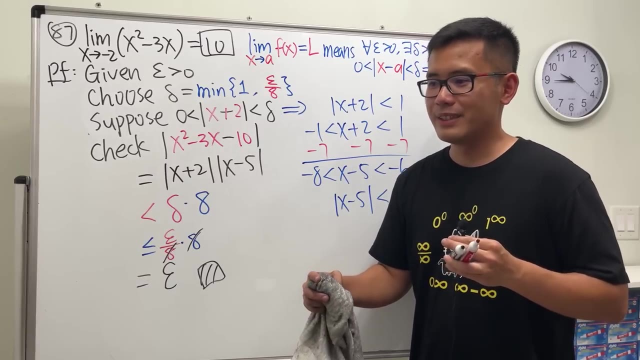 and it will still work. theoretically speaking, yeah, but to really understand what's going on for epsilon delta definition, i will highly recommend you guys to watch my video, because i use my actual example, my actual numbers and also the graph, and i explained it when i'm like when i was like 100 percent energy- right now i don't know. 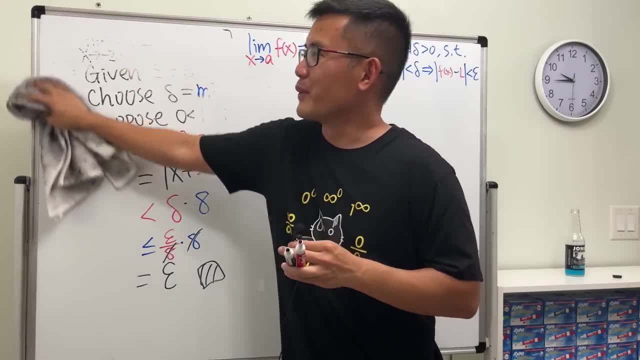 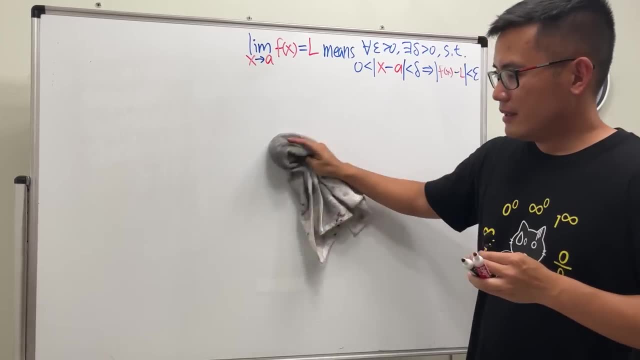 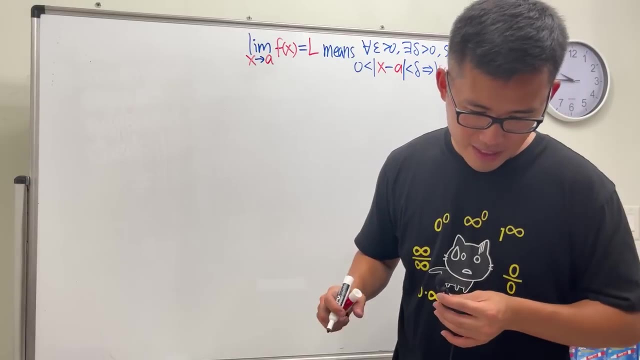 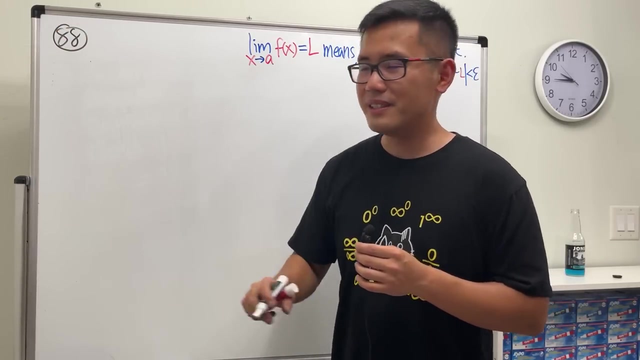 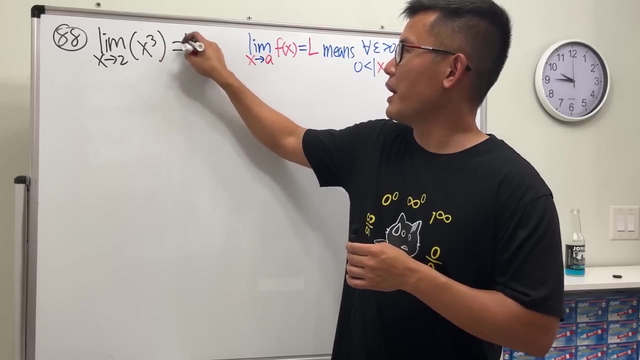 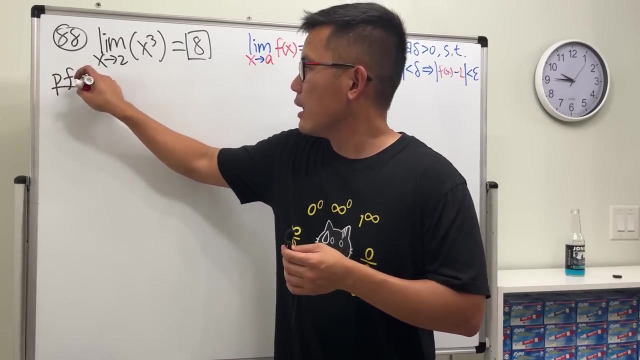 i. i use 78 of my life already, so i have like 13 percent more. okay, all right. now, i love cubic example. i also picked this one on purpose number 88: what's a limit as x approaching 2 of x to the third power? you know it's 8.. y, look 88 and an 8. okay, all right, proof. 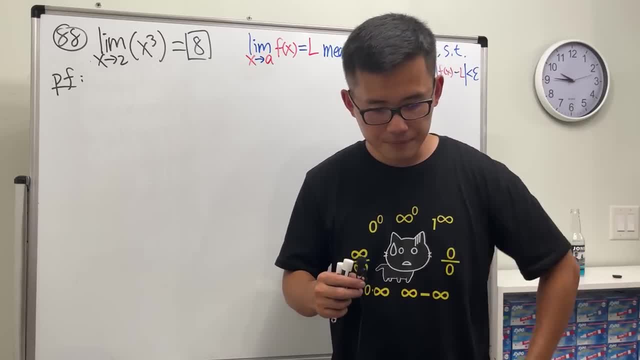 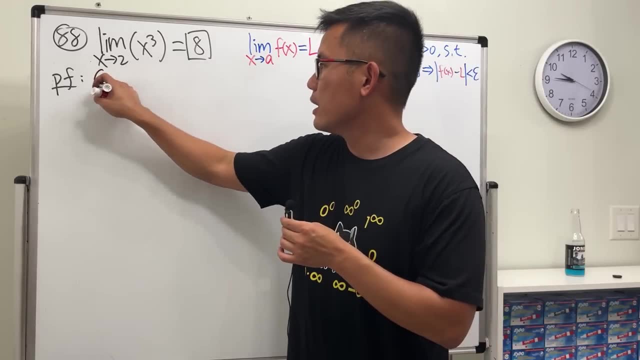 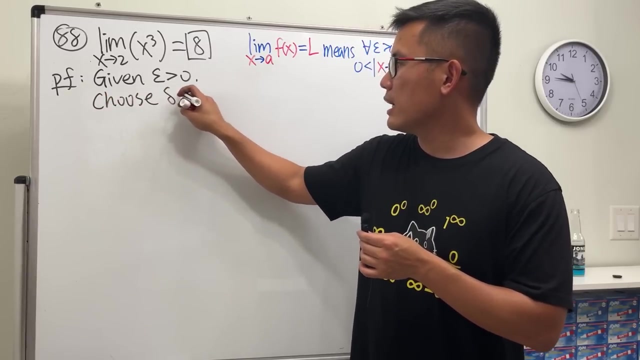 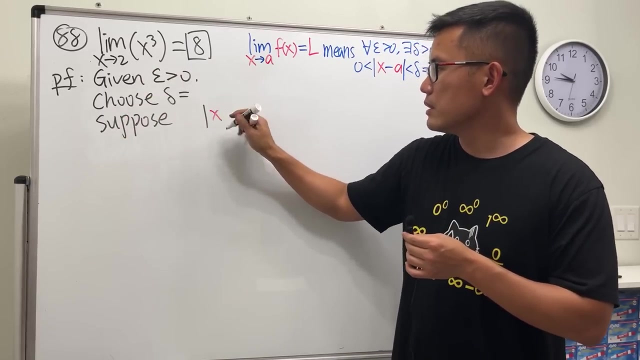 this is like extension of the quadratic case, if you have understood? uh, the quadratic cases, they change all the time than this right here. not so bad, By the way. given epsilon greater than 0, choose Delta. I don't know. yet suppose epsilon for u of x minus 2 is less than Delta, and 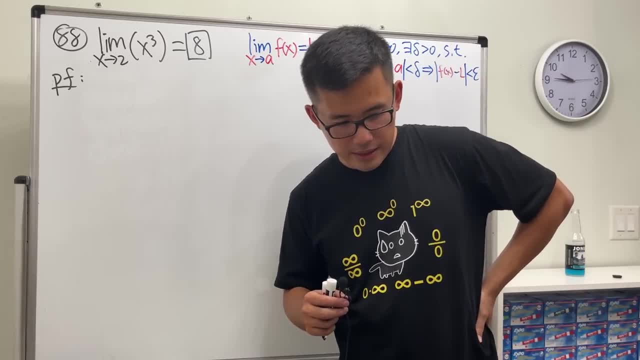 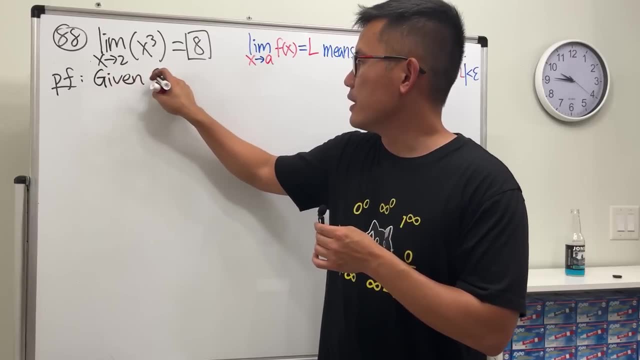 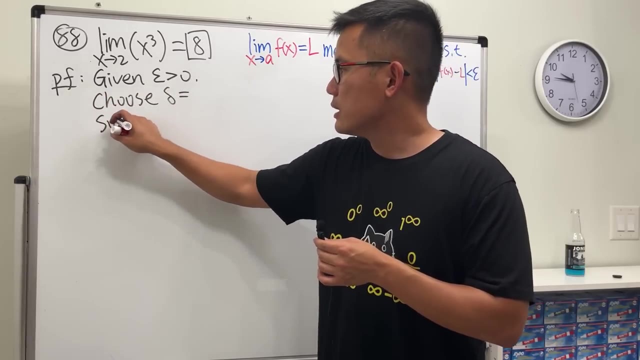 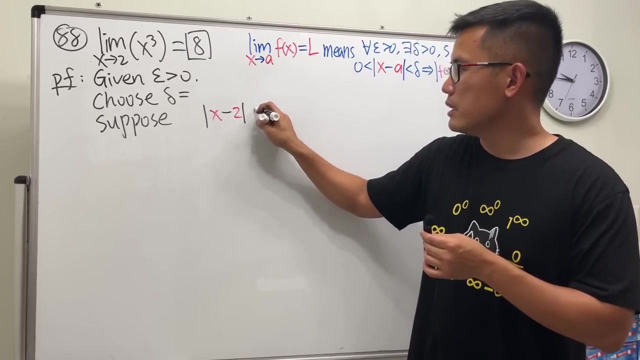 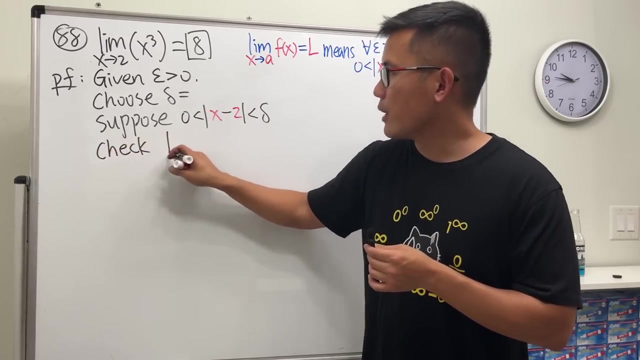 understood the quadratic cases. then this right here. not so bad, by the way. given epsilon greater than 0, choose delta. I don't know yet. suppose absolute value of x minus 2, ok, is less than delta. and put this: check: absolute value function minus the limit. alright, here we go. 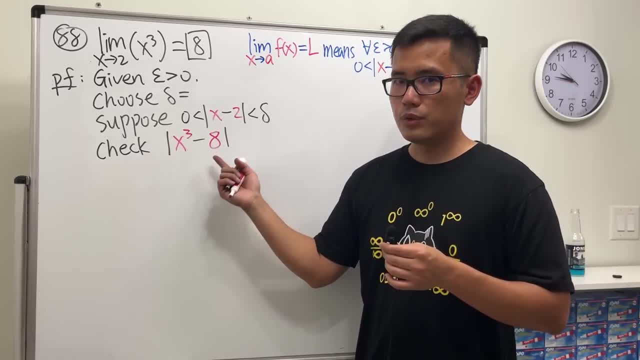 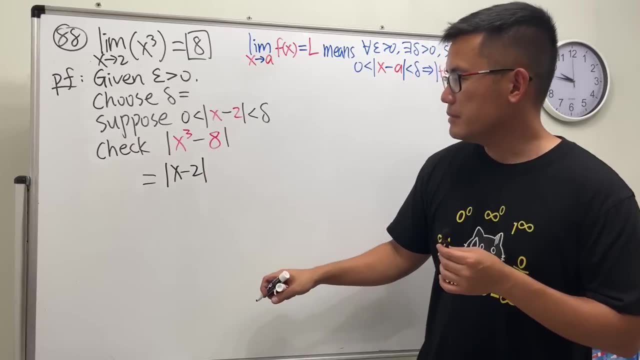 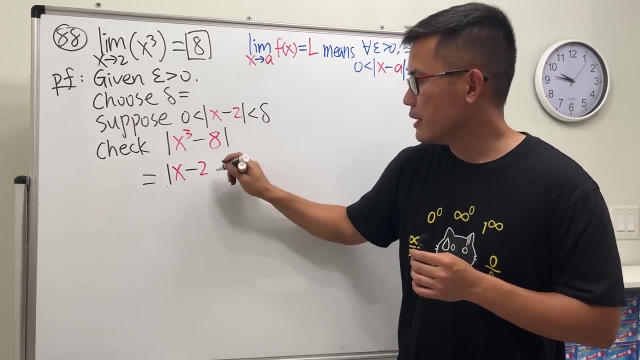 algebra work. this is the difference of two squares. this is the same as 2 to the third power. so we can factor this as absolute value of x minus 2 times absolute value of x minus 2 times x square plus 2 times x, which is just 2x. 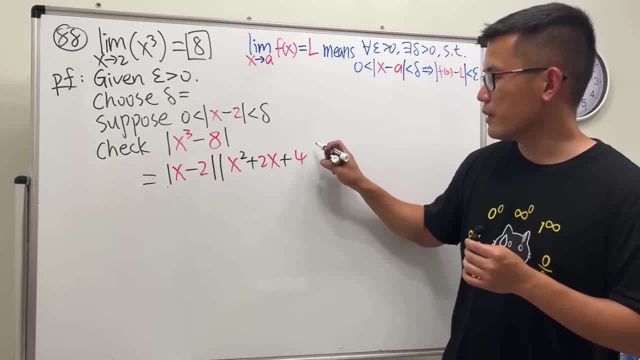 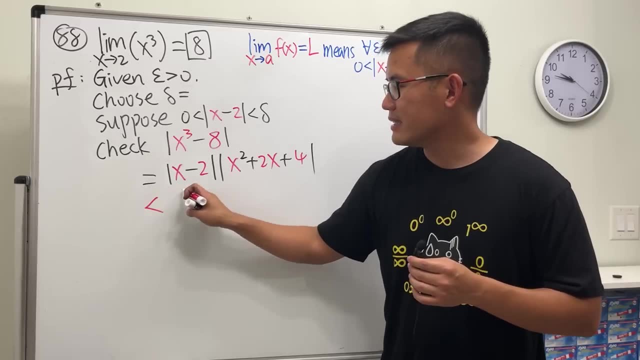 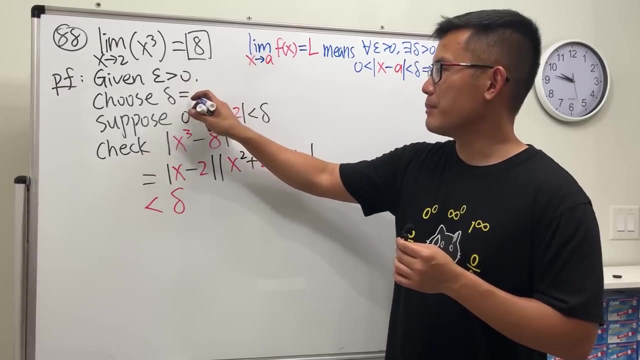 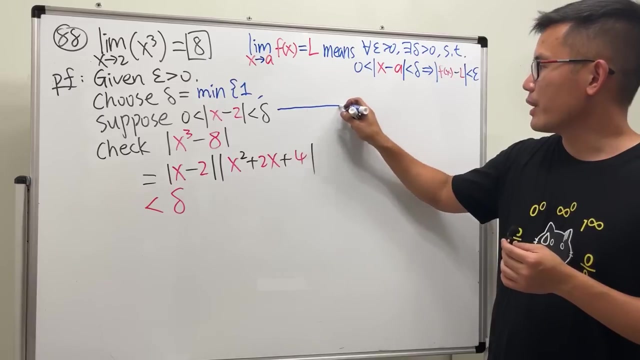 and lastly, we add 2 square, which is 4. cool, what's this? this is good. yeah, less than delta. everybody likes it. what's that? don't worry, come back to the delta part. and then we just say: let's use 1. ok, starting right here. 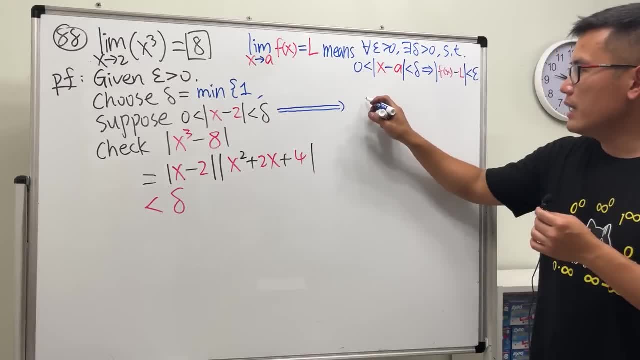 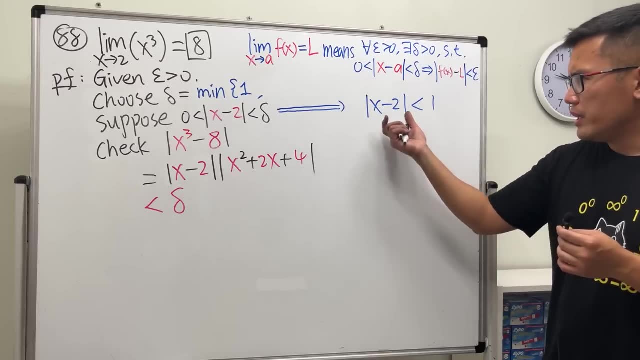 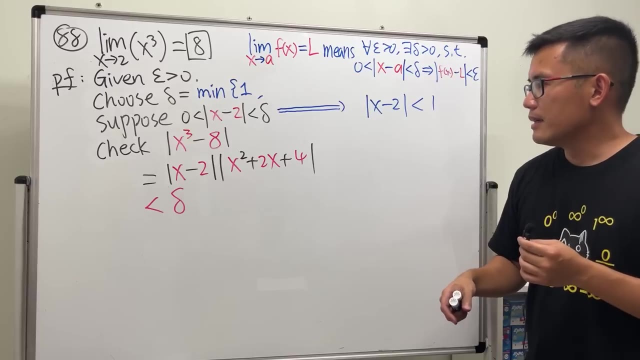 let's draw this a little bit longer. ok, so we are looking at absolute value of x minus 2 is less than 1, for here we want to get to x square part, so it's a little bit tricky, so pay attention right here, but the idea is the same. 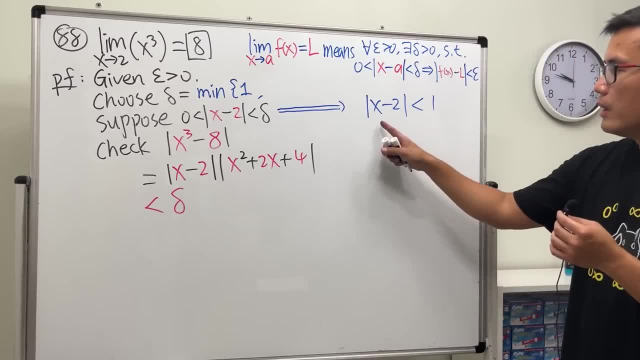 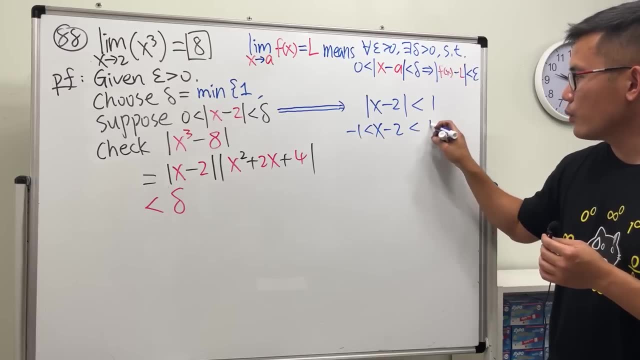 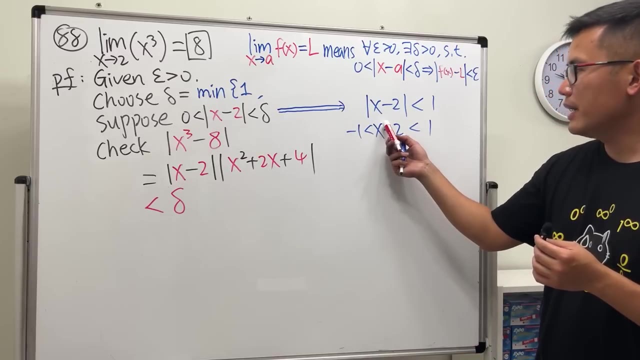 if you can get a bound for this, you are in good shape anyway. so let's do this. so we get x minus 2 is in between of negative 1 and 1, and for this particular case I'm going to, just because I cannot get to. 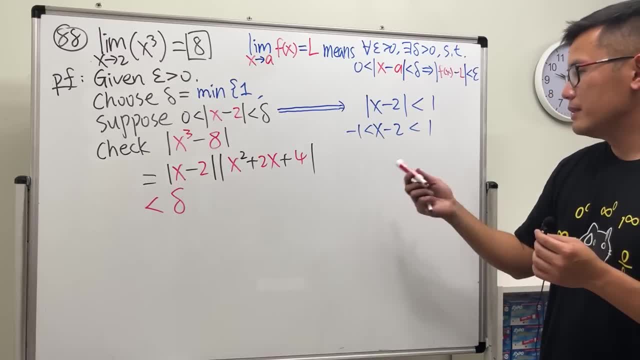 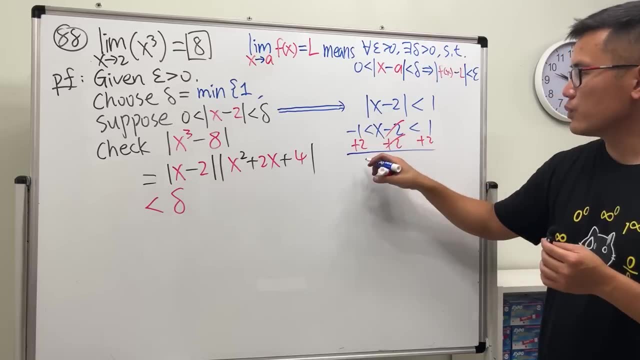 x square, unless I square everybody. no, let's not do that. let's just add 2 to everybody, you'll see why. so they cancel. and then we see this is 1, this is x and this is 3, and then, as I told you earlier, we can say: 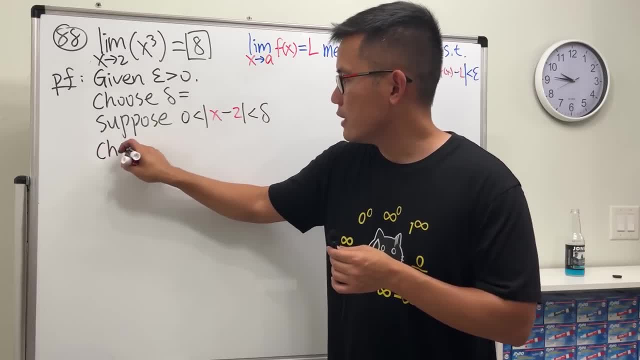 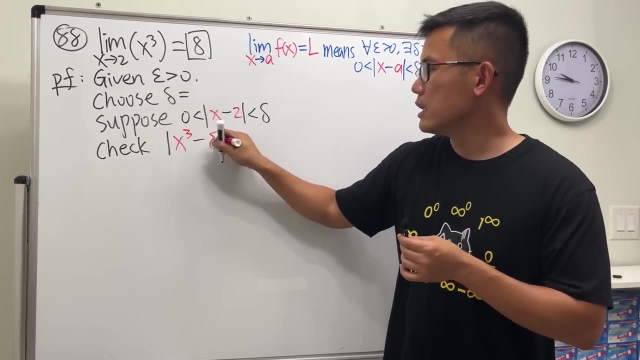 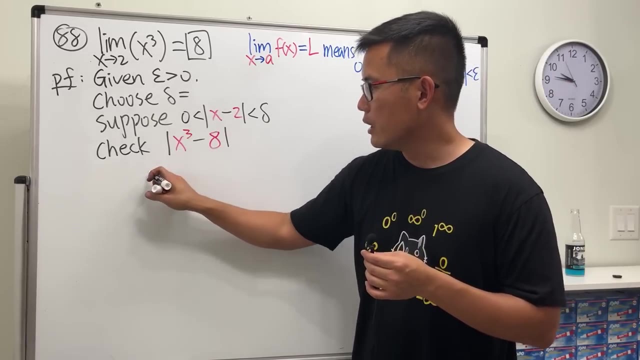 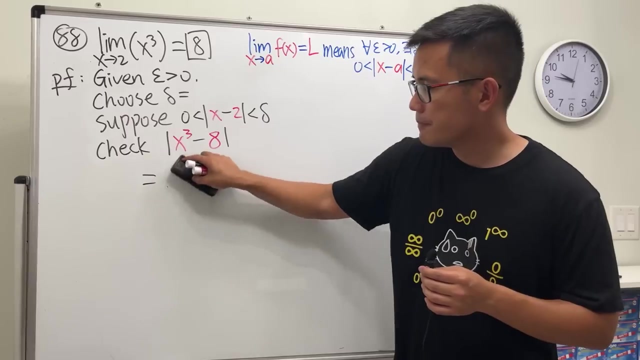 put this check: epsilon for u function minus the limit. all right, here we go, algebra work. This is the difference of two squares. this is the same as 2 to the third power. so we can factor this as epsilon for u of x minus 2 times epsilon for u of x minus 2. 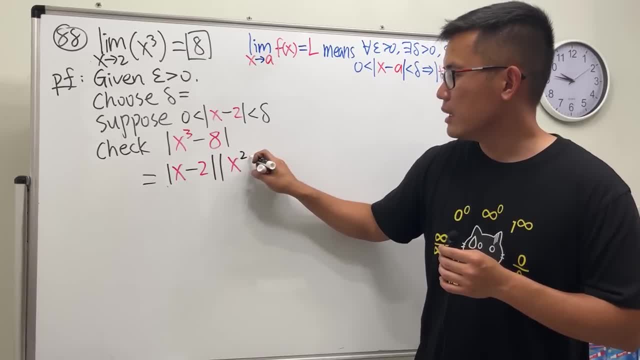 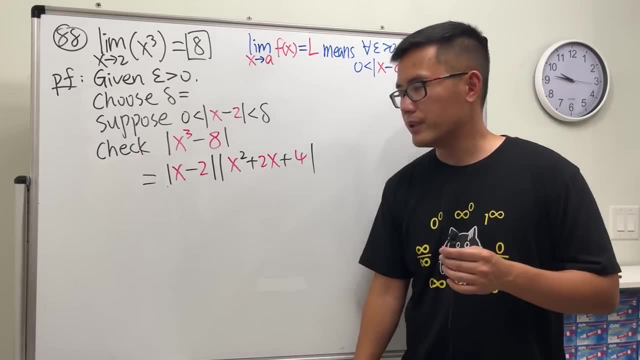 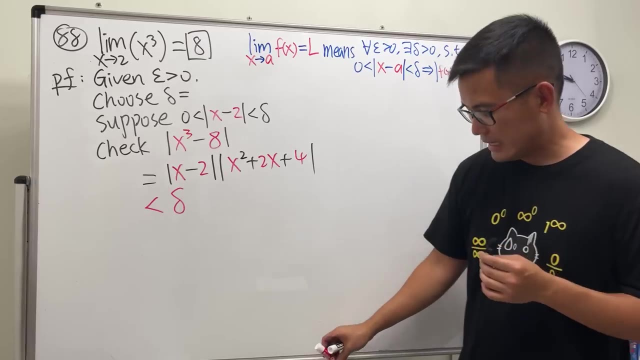 times epsilon for u of x minus 2 times x squared plus 2 times x, which is just 2x. and lastly, we add 2 squared, which is 4.. Cool, What's this? This is good, Yeah, less than Delta. Everybody likes it. What's that? 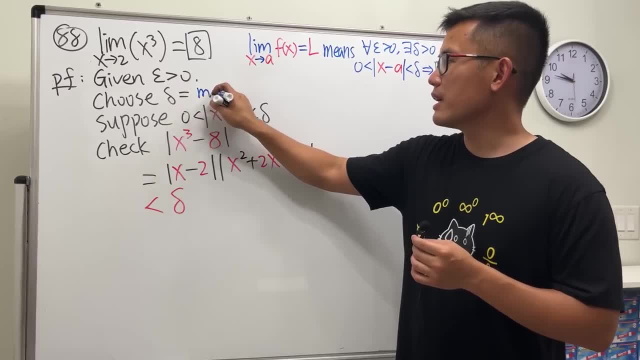 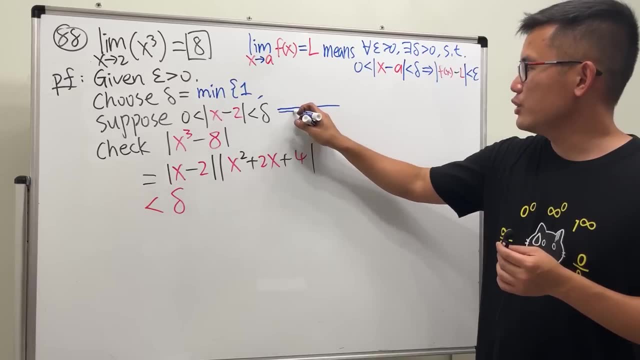 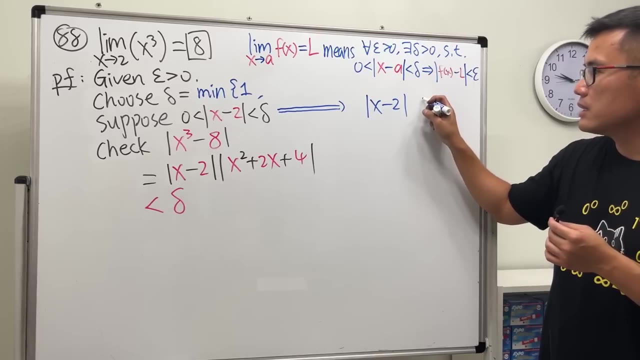 Don't worry, Come back to the Delta part, and then we just say: minimum, let's use 1.. Okay, starting right here, let's draw this a little bit longer. We'll just draw this a little bit longer. Okay, so we're looking at absolute value of x minus 2 is less than 1.. For here we want: 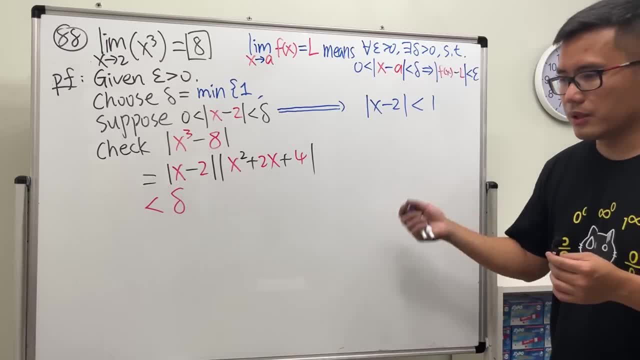 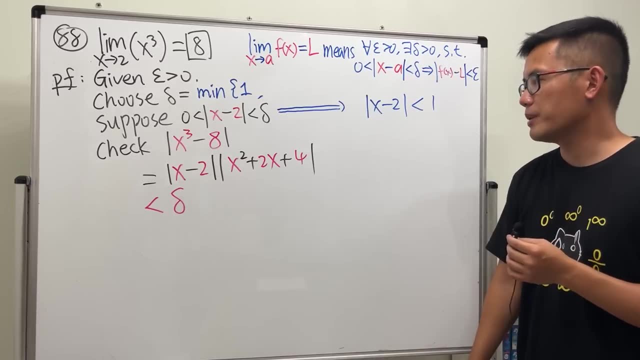 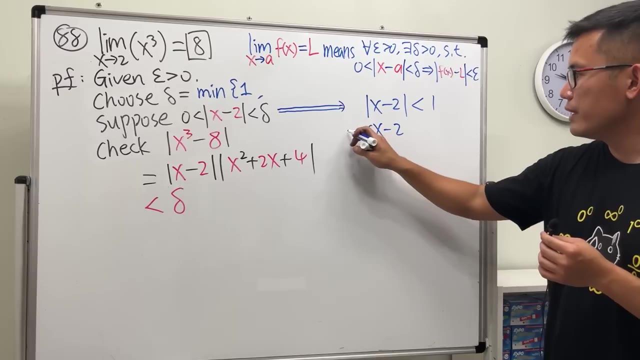 to get to x squared part. so it's a little bit tricky, so pay your attention right here, but the idea is the same. If you can get a bound for this, then you are in good shape. Anyway, open this so we get x minus 2 is in between negative 1 and negative 1.. 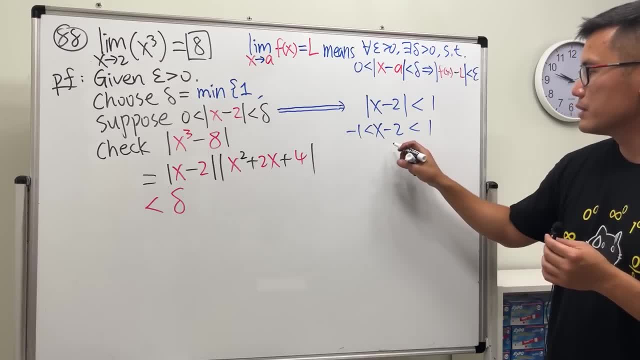 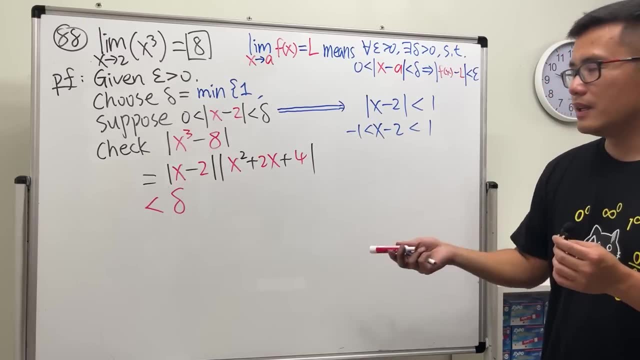 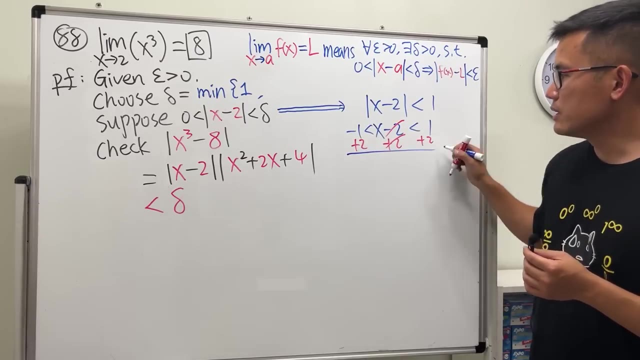 And for this particular case I'm going to, just because I cannot get to x squared unless I square everybody. No, let's not do that, Let's just add 2 to everybody, You'll see why. So they cancel. and then we see: this is 1, this is x and this is 3.. 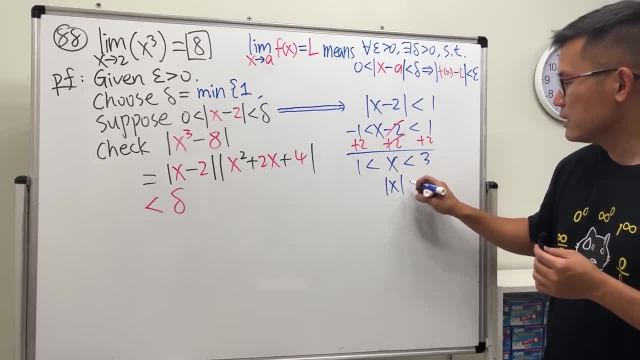 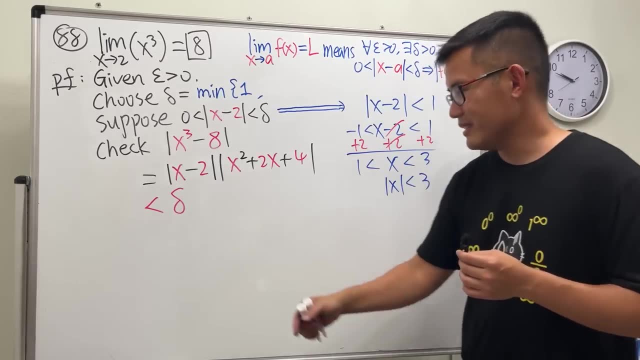 And then, just like what we did earlier, we can say: absolute value of x is less than 3.. So you pick the bigger absolute value, which is this. Now, here is the deal. We have this condition thanks to that, and we want to see this. 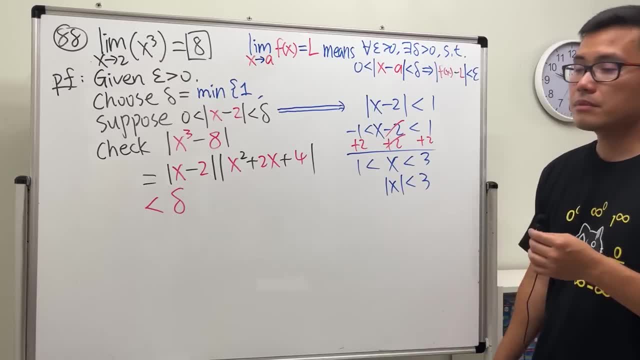 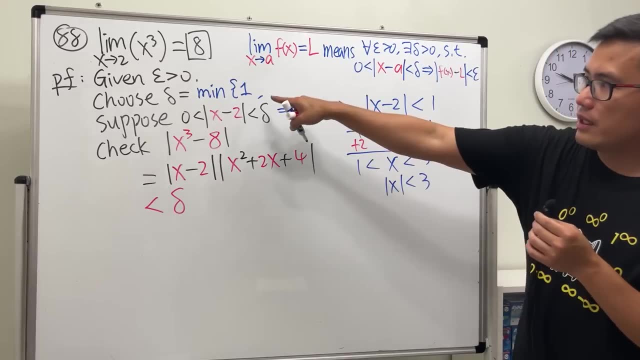 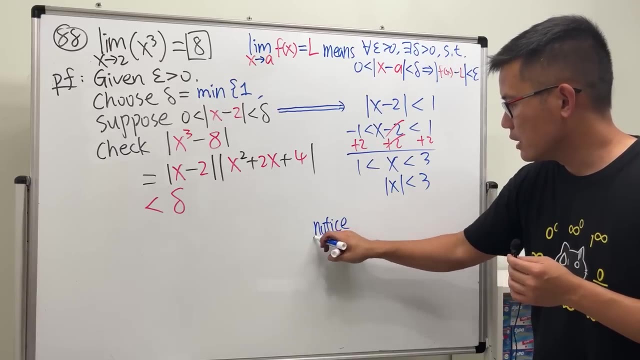 absolute value of x is less than 3, so you pick the bigger absolute value, which is this. now, here is the deal. we have this condition thanks to that and we want to see this. so I will just tell you guys that notice from here and there we are going to make a connection. 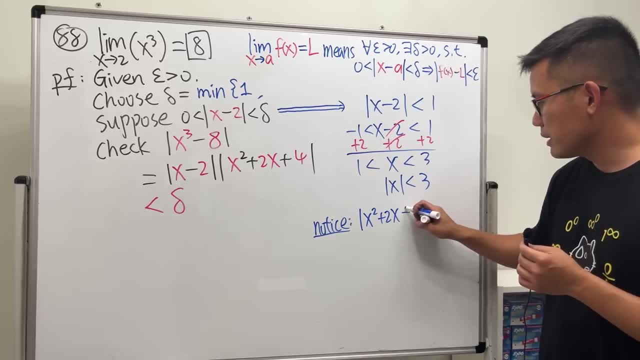 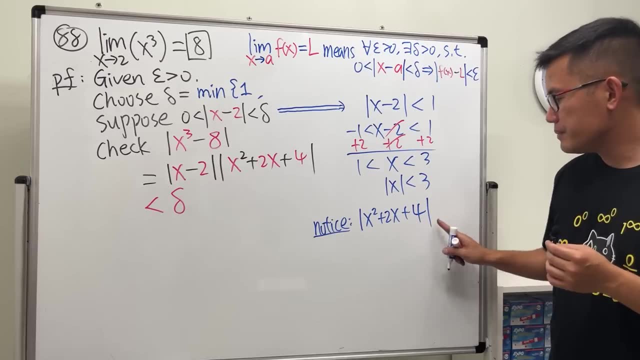 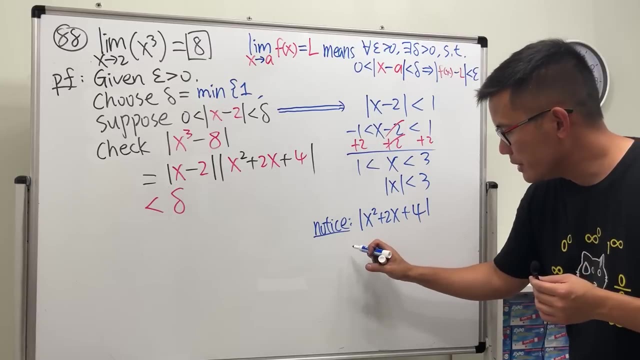 when we have the absolute value of x square plus 2x plus 3 plus 4, you see how we have the absolute value of the sum. this, right here, is going to be guaranteed: less than or equal to the absolute value of the first plus the absolute value of the second. 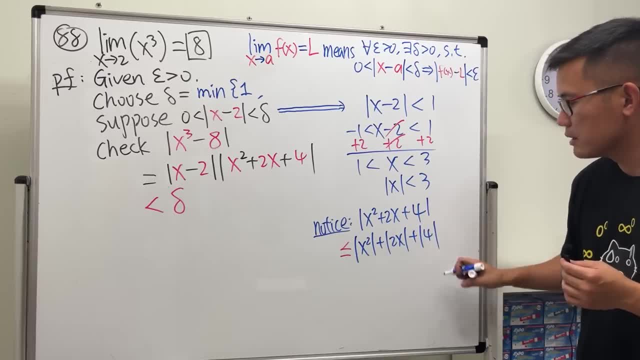 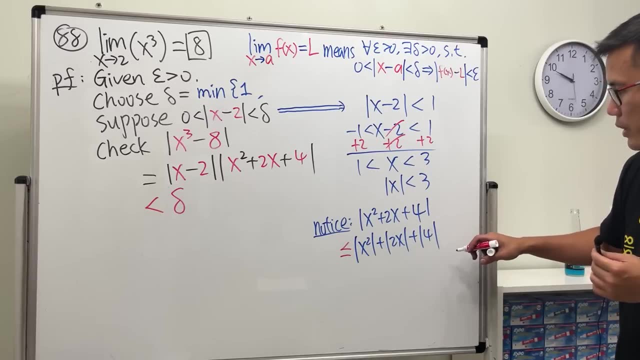 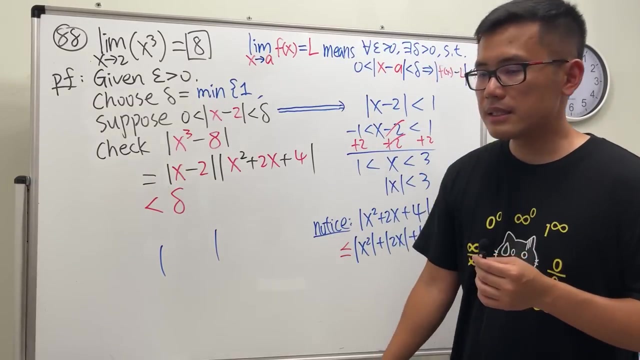 plus the absolute value of the third. yeah, so this is like the extent version of the so called triangle inequality. so let me just write it down somewhere by triangle in equality. let me give you guys an example real quick. suppose you have absolute value. let's say we have. 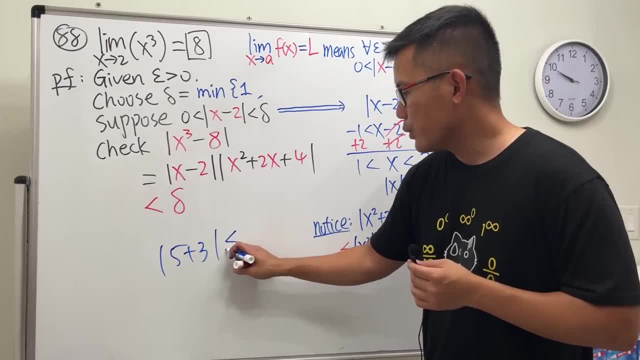 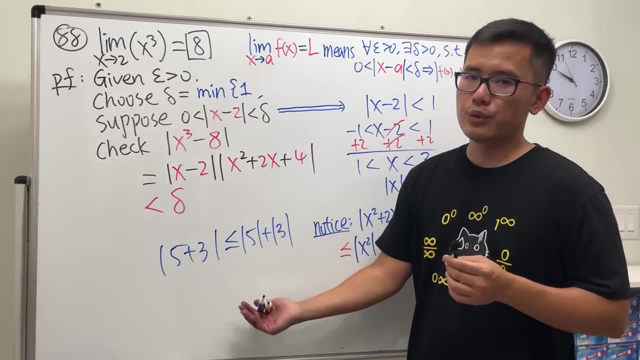 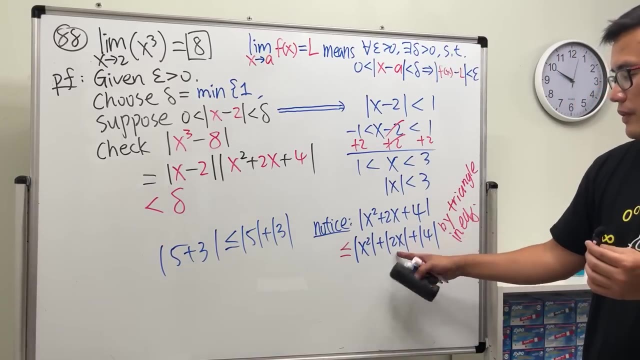 5 plus 3. well, is this less than or equal to absolute value of 5 plus absolute value of 3? yes, in fact they are equal, because it's 8. it's actually equal to 8, but if you have, let's say this because you don't know if x is negative. 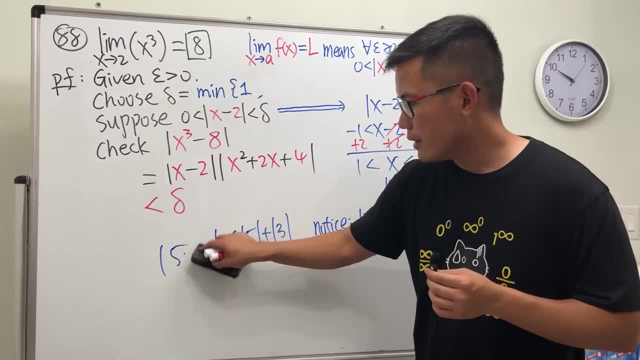 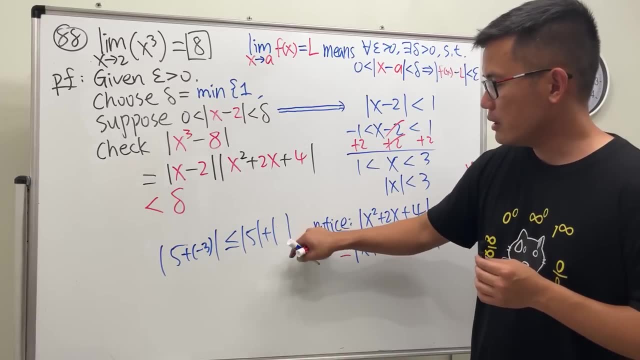 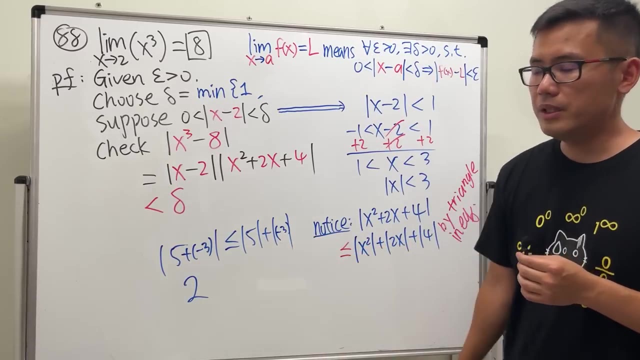 or not, i don't know right. so let's say, if we have 5 plus negative 3, i'm going to put this 3 right here and make it negative 3. you see, here we actually just get 2, but then here we have 8. the right hand side is bigger. 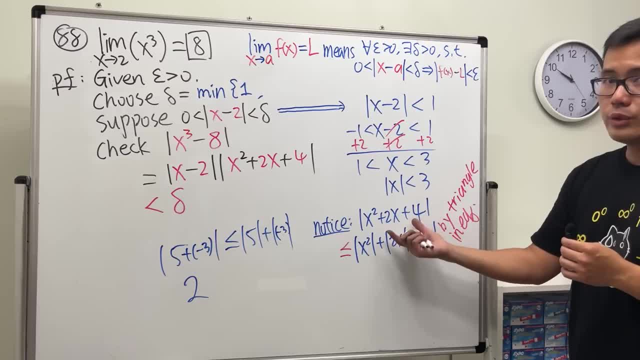 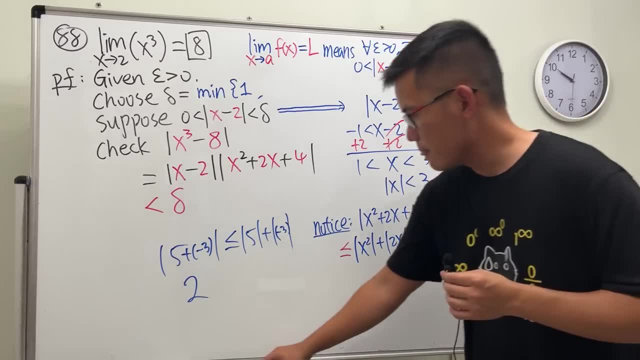 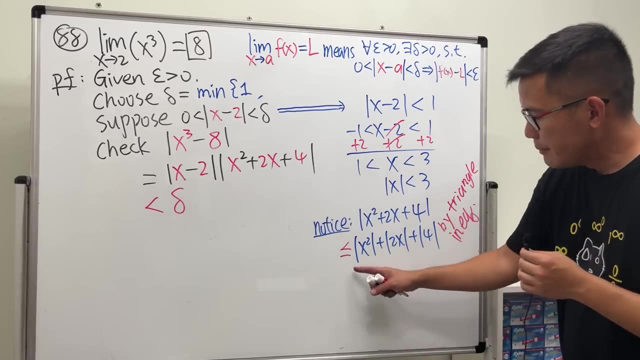 so, again, when we have absolute value of a sum, this right here is less than or equal to the sum of the absolute values. this is the so called triangle inequality. so that's another thing that you'll keep in mind, because once we have this, check this out, i'm going to use 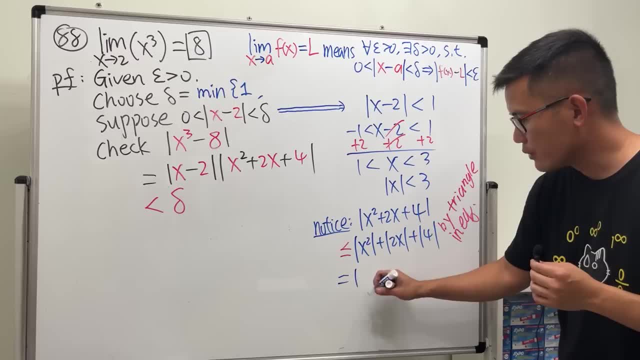 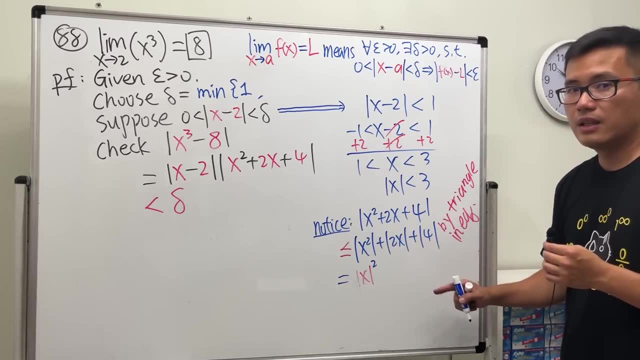 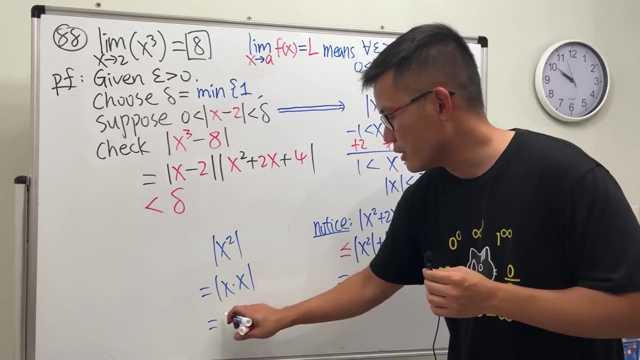 equal sign, because this is equal to absolute value of x. this right here, is equal to absolute value of x square. we can put a square on the outside and the reason for that is absolute value of x square is equal to absolute value of x times x and per our discussion earlier, 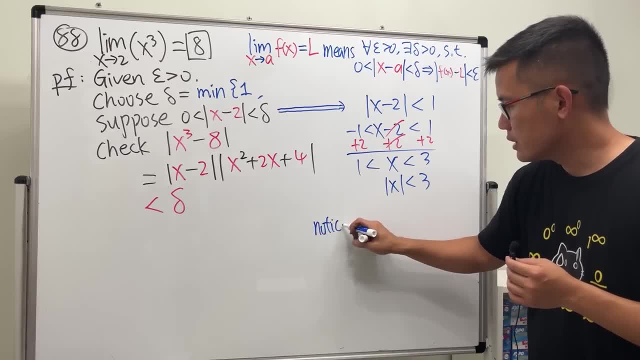 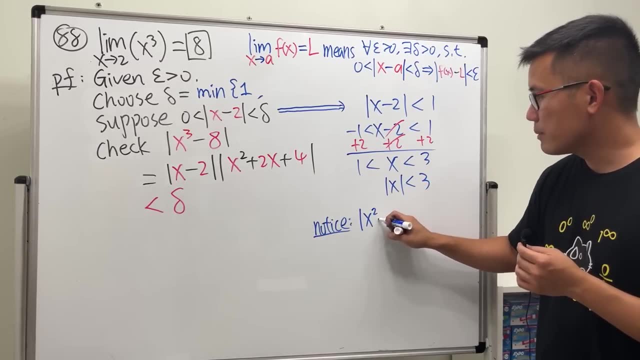 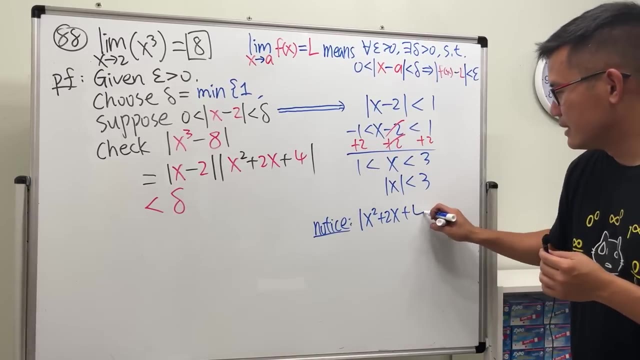 So I will just tell you guys that notice from here and there we are going to make a connection. When we have the absolute value of x squared plus 2x plus 3, that's plus 4.. You see how We have the absolute value of the sum. 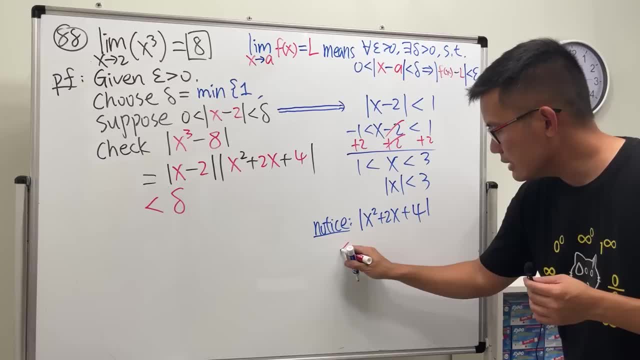 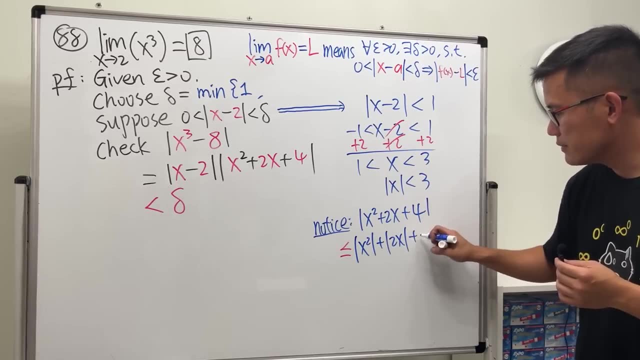 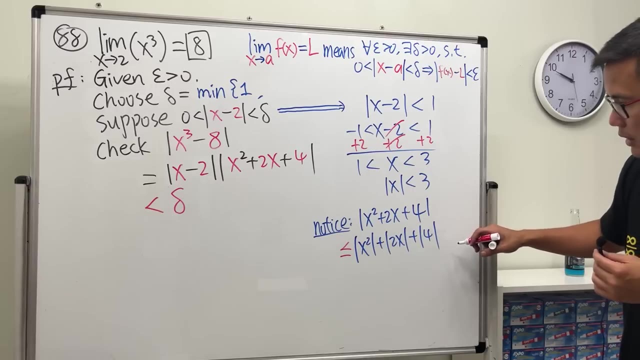 This right here is going to be guaranteed: less than or equal to the absolute value of the first plus the absolute value of the second plus the absolute value of the third. Yeah, So this is like the extended version of the so-called triangle inequality. So let me just write it down somewhere. 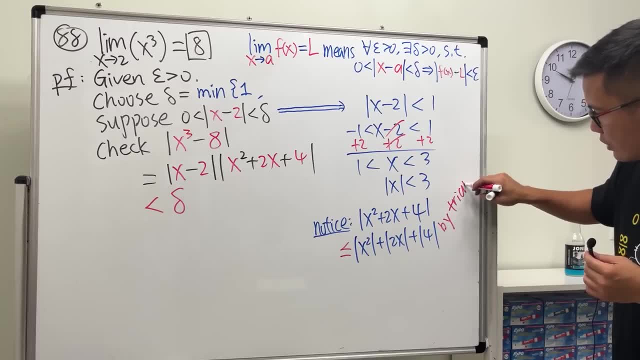 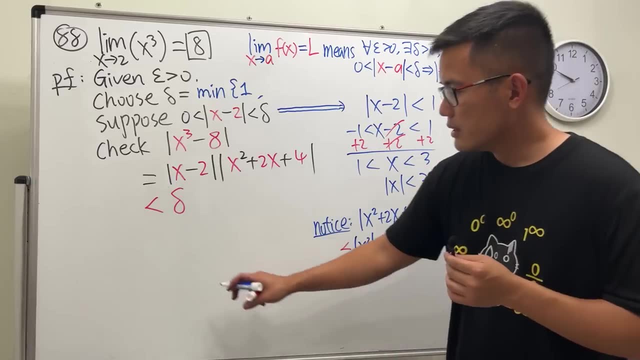 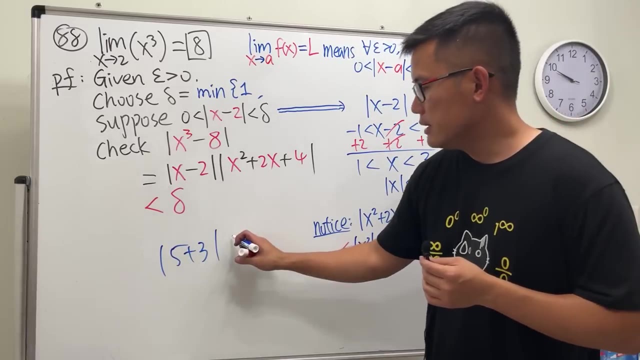 By triangle: inequality, Inequality. Let me give you guys an example real quick. Suppose you have absolute value. Let's say we have 5 plus 3.. Well, is this less than or equal to absolute value of 5 plus absolute value of 3?? 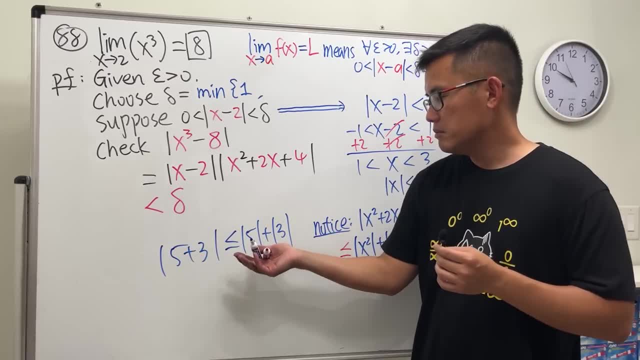 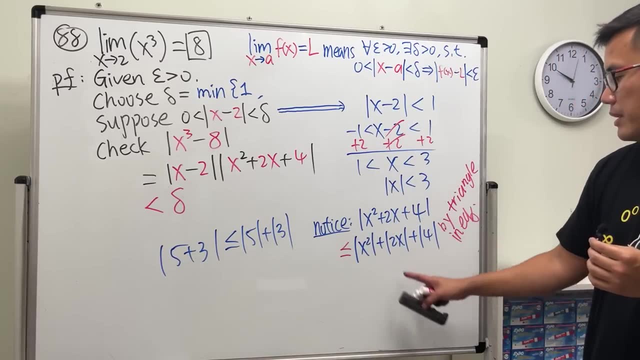 Yes, In fact they are equal because it's 8.. It's actually equal to 8.. But if you have, let's say this, Because you don't know if x is negative or not, I don't know right. 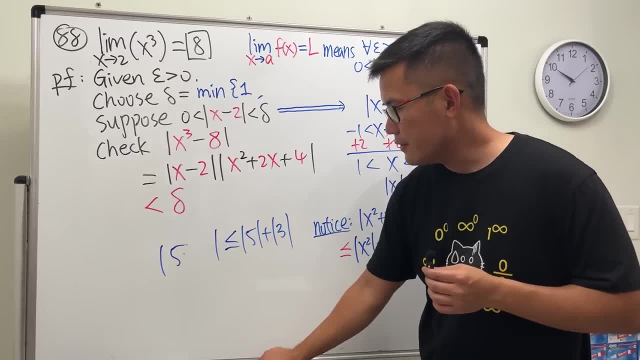 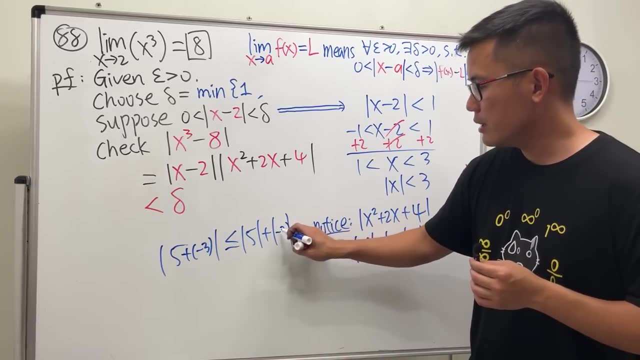 So let's say, if we have 5 plus negative 3.. I'm going to put this 3 right here and make it negative 3.. You see, here we actually just get 2, but then here we have 8.. The right hand side is bigger. 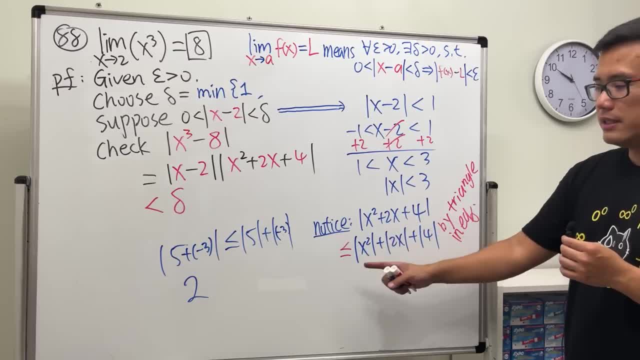 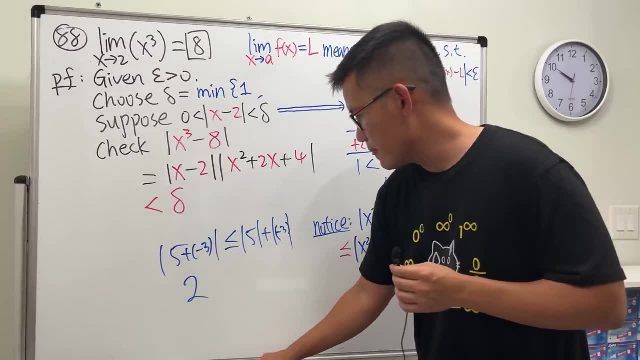 So, again, when we have absolute value of a sum, this right here is less than or equal to the sum of the absolute values. This is the so-called triangle inequality. So that's another thing. So that's another thing that you'll keep in mind. 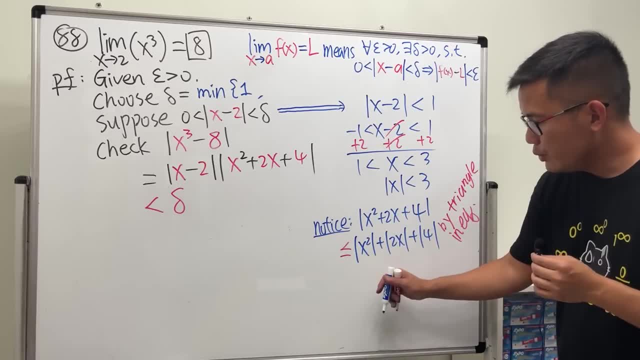 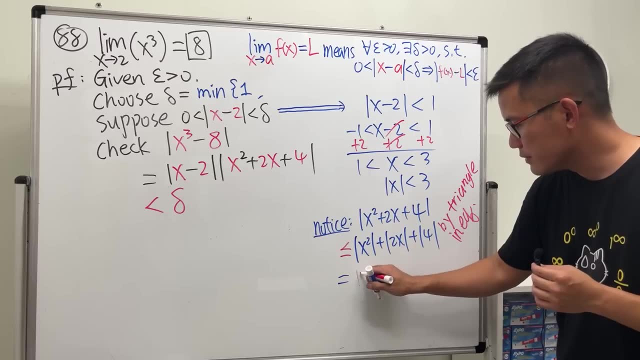 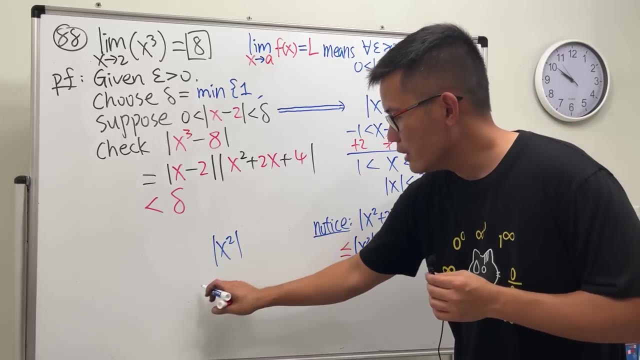 Because once we have this, check this out, I'm going to use equal sign, because this is equal to absolute value of x. This, right here, is equal to absolute value of x squared. We can put a square on the outside And the reason for that is: absolute value of x squared is equal to absolute value of x times x. 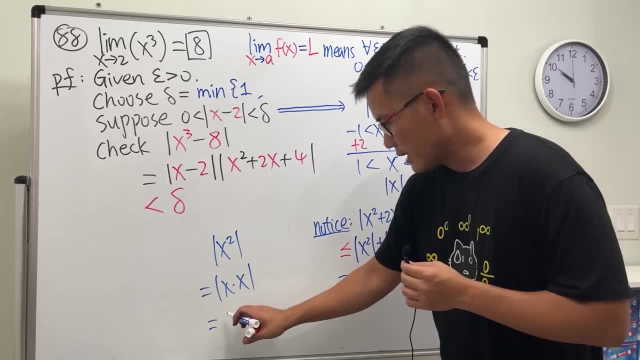 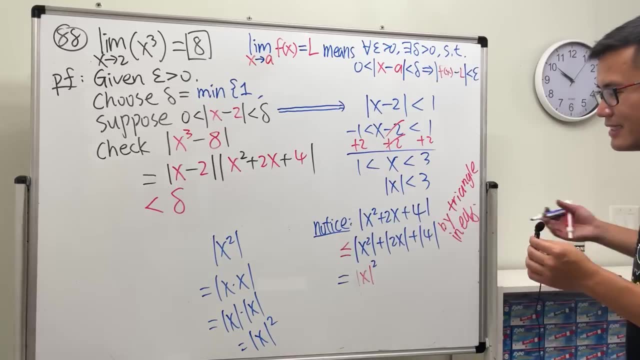 And in our discussion earlier, the absolute value of a product is a product of the absolute value. So this is the same. It depends if you guys have seen this kind of proof or not in your class. Hopefully you can just go from here to here. 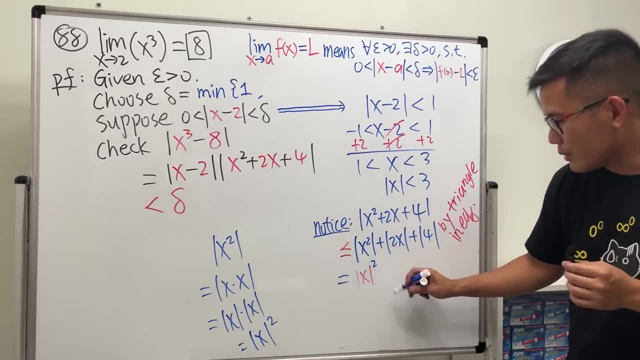 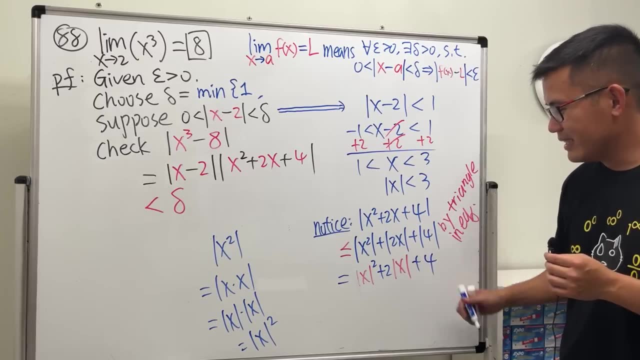 But anyway it's this equal sign And then you can put a 2 on the outside, So it's plus 2, absolute value of x And then absolute value of 4 is just 4.. So from here to here it's just straightforward equal sign. 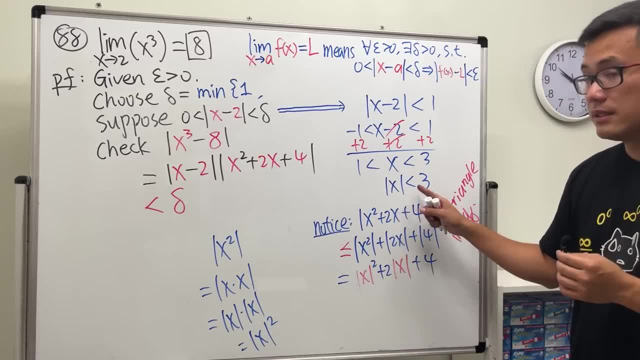 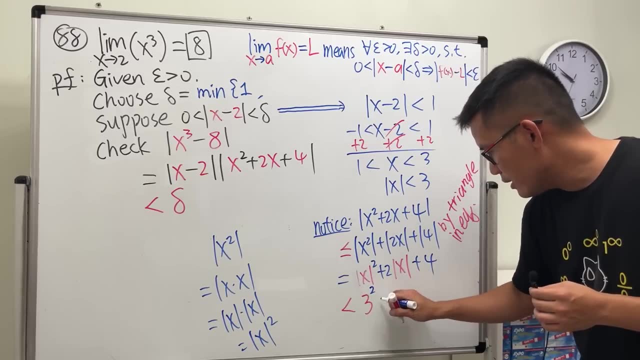 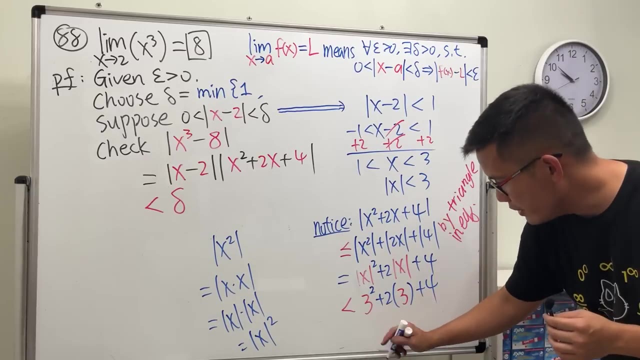 Now we know absolute value of x is less than 3.. So we can replace the real absolute value with less than, And then 3 squared plus 2 times 3.. And then plus 4.. And then from here to here it's going to be equal sign, because it's just computation. 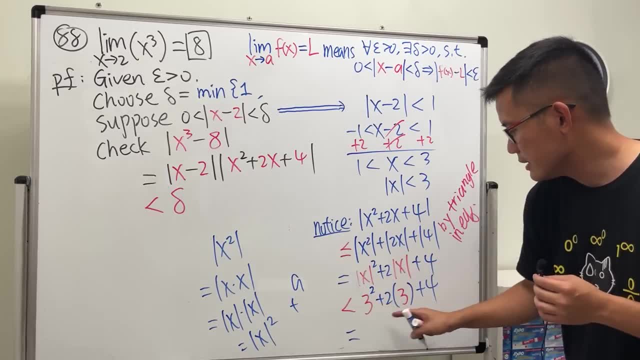 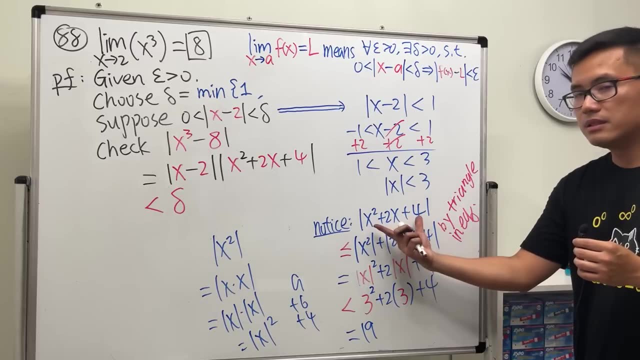 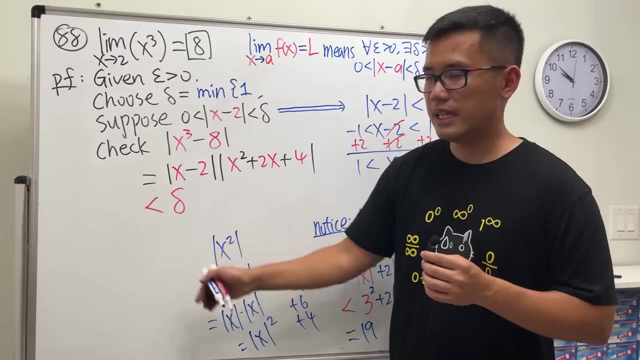 And let's see, This is 9 plus 6 plus 4.. So 19.. So, all in all, we are saying that this absolute value of expression is less than 19,. which is exactly what we want. This is less than 19.. 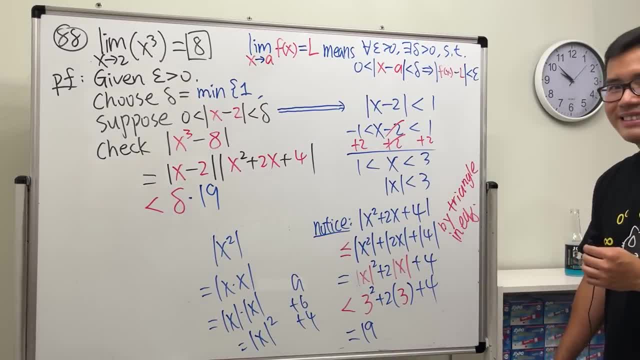 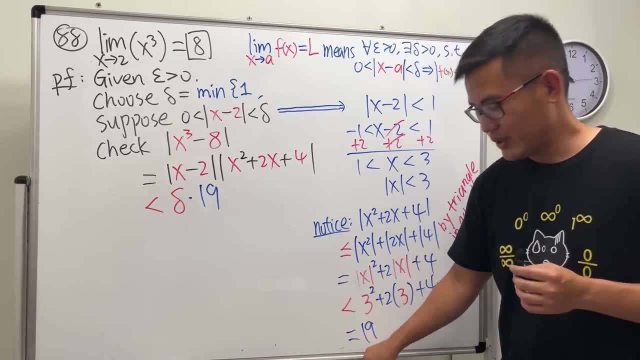 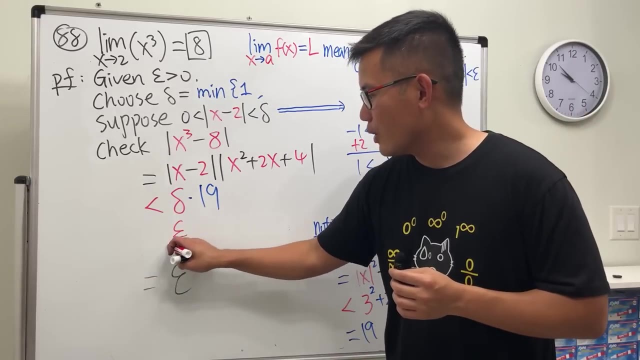 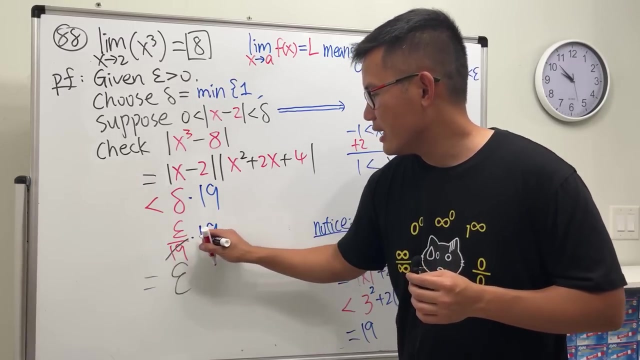 Let's have a look, Because you know, once you have that, we're almost done. At the end you want epsilon Delta shall be epsilon over 19.. That way when we multiply by 19, they cancel. So we can come back here and say we also need epsilon over 19.. 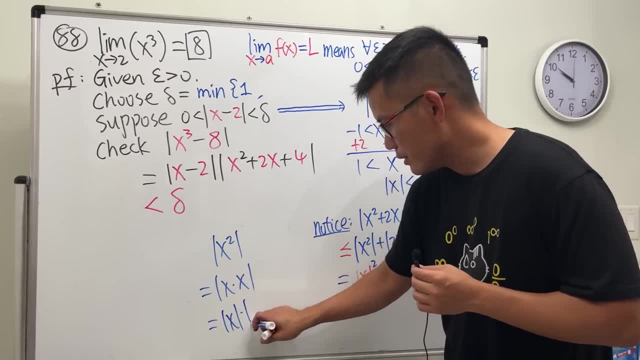 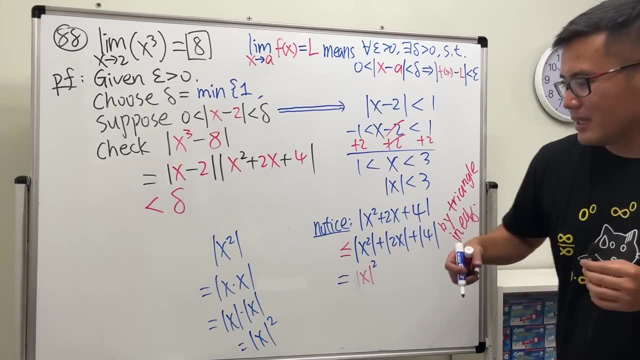 the absolute value of a product is a product of the absolute value. so this is the same, as it depends if you guys have seen this kind of proof or not in your class. hopefully you can just go from here to here, but anyway, it's this equal sign. 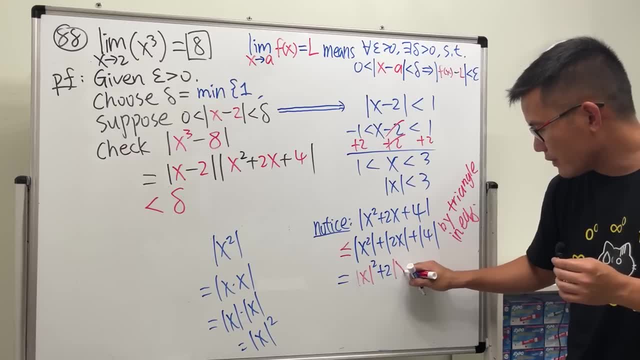 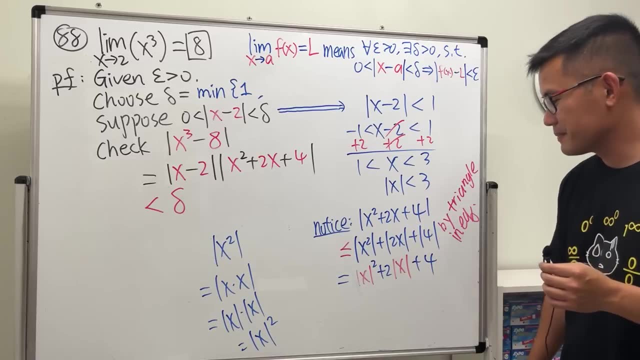 and then you can put a 2 on the outside, so it's plus 2 absolute value of x and then absolute value of 4 is just 4. so from here to here is just straight forward: equal sign. now we know absolute value of x is: 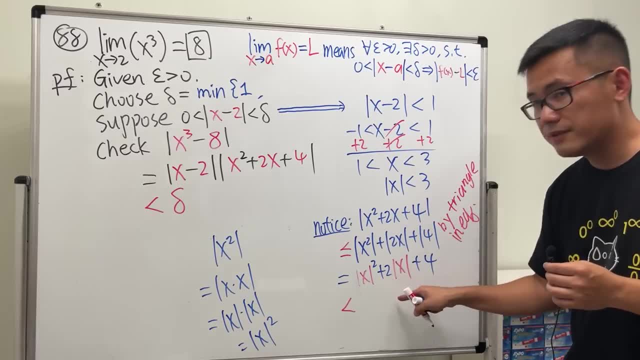 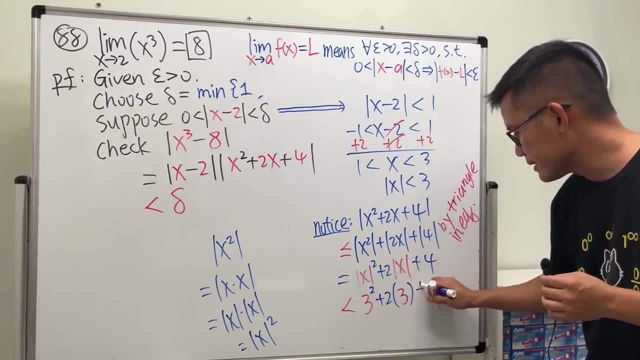 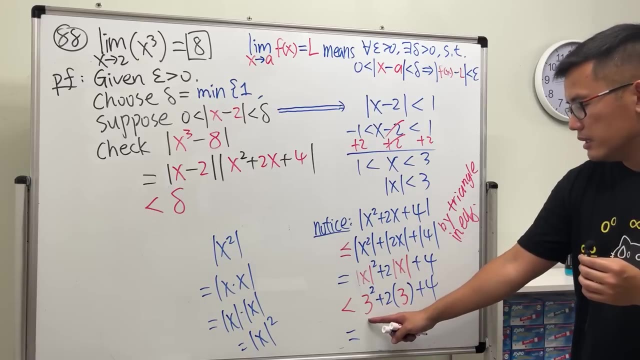 less than 3, so we can replace the real absolute value with less than, and then 3 square plus 2 times 3, and then plus 4, and then from here to here it's going to be equal sign, because it's just computation. and let's see, this is: 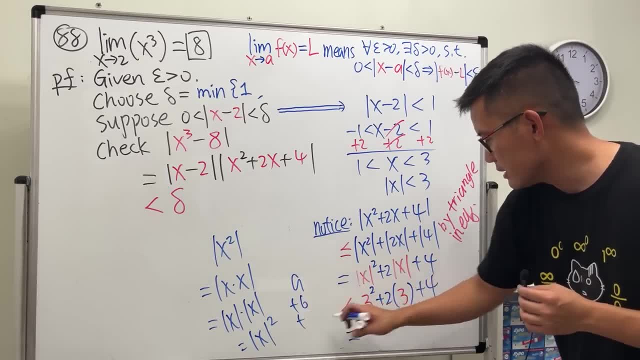 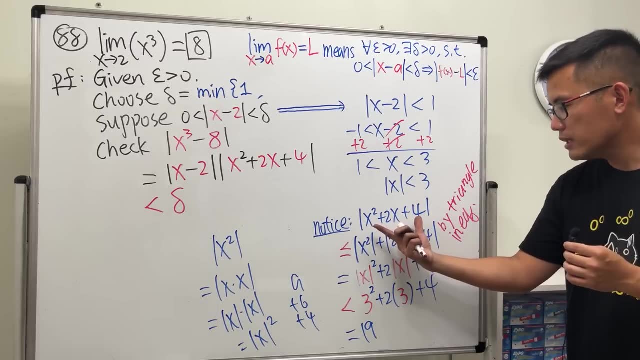 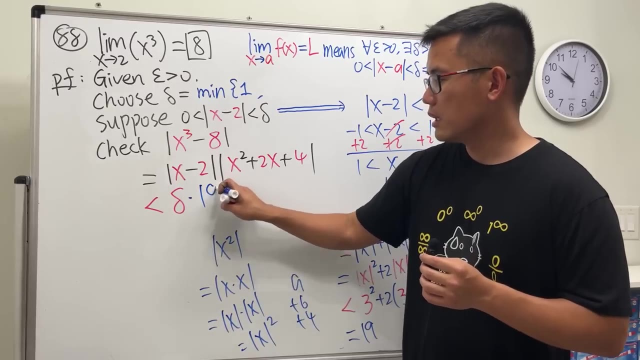 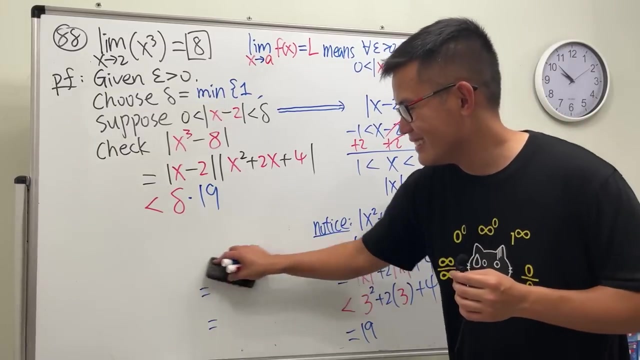 9 plus 6 plus 4, so 19. so all in all, we are saying that this absolute value of expression is less than 19, which is slightly 1. this is less than 19. let's have a look, because you know, once you have that. 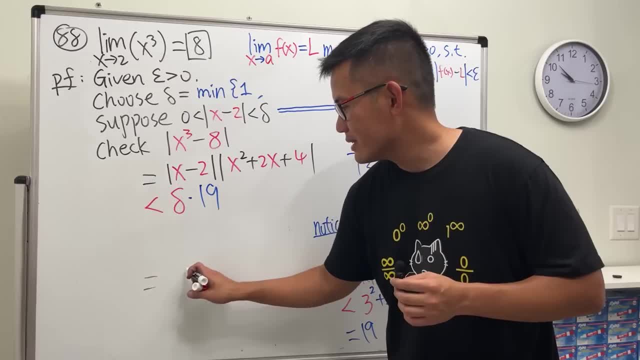 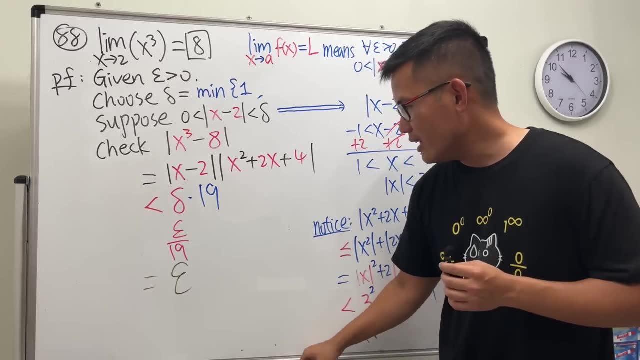 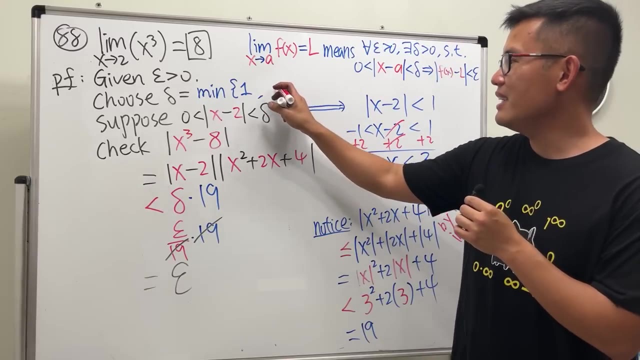 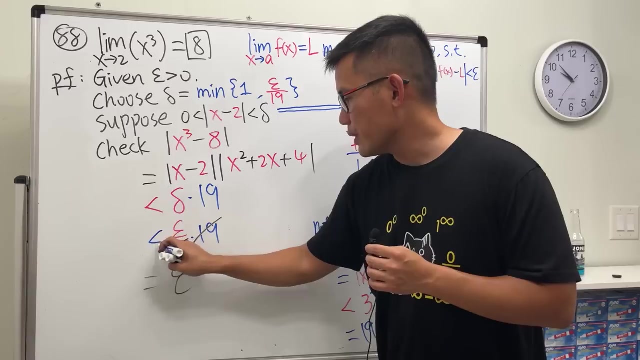 we are almost done. at the end you want epsilon delta shall be epsilon over 19. that way when we multiply by 19 they cancel. so we can come back here and say we also needed epsilon over 19 and close this less than or equal to. finally, don't you ever. 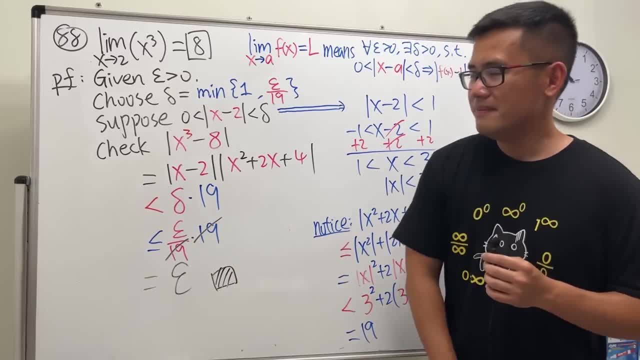 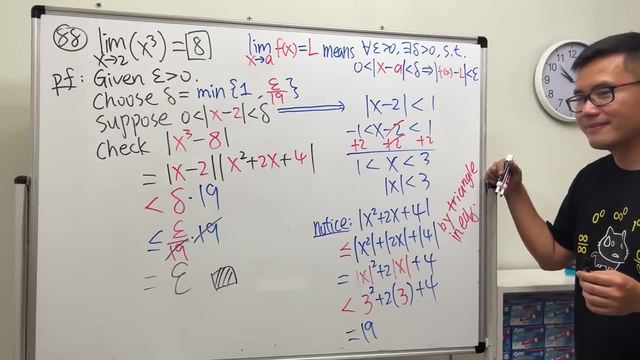 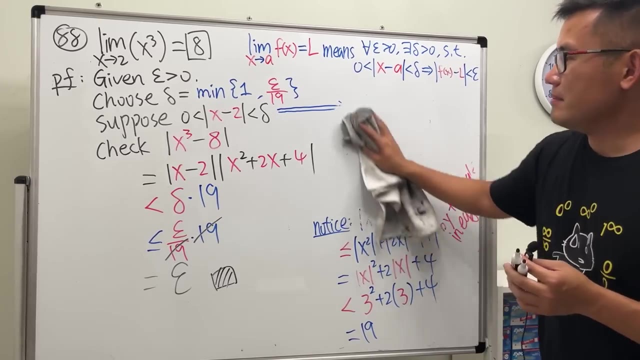 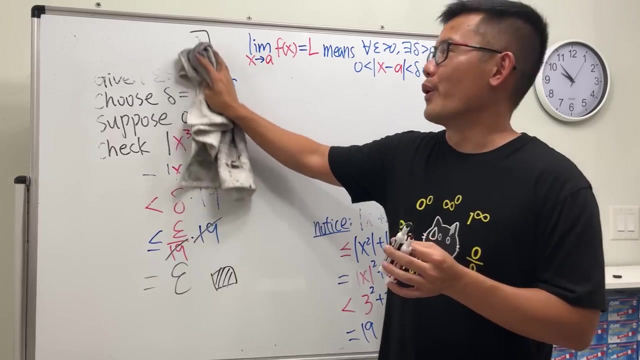 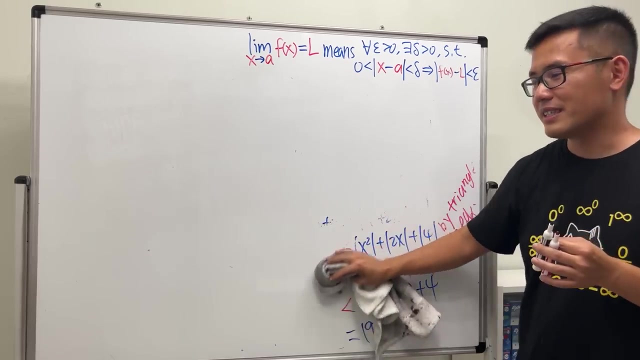 forget the box shading. ah, cool. absolute, I mean. um, epsilon delta definition is a lot of fun when you know how to work it out, when you know how to write down a good proof for it. it's it feels very satisfying, feels very, very satisfying. yeah, I think this is the reason why. 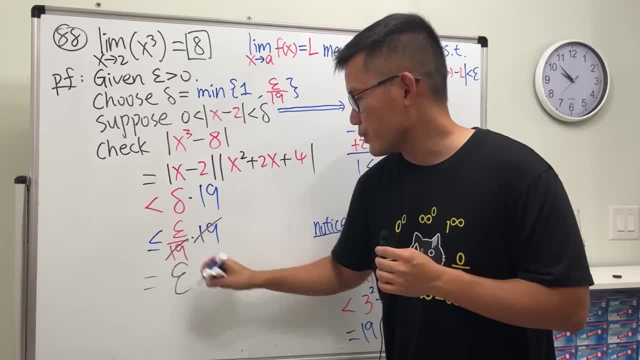 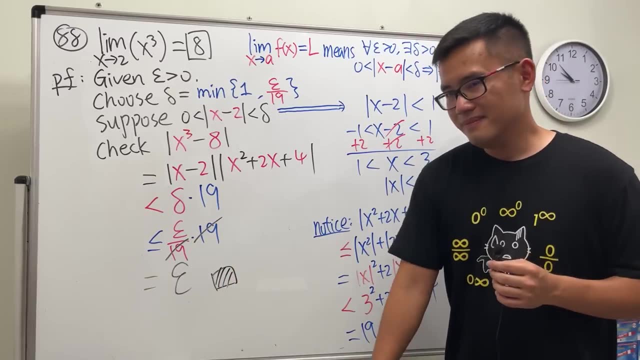 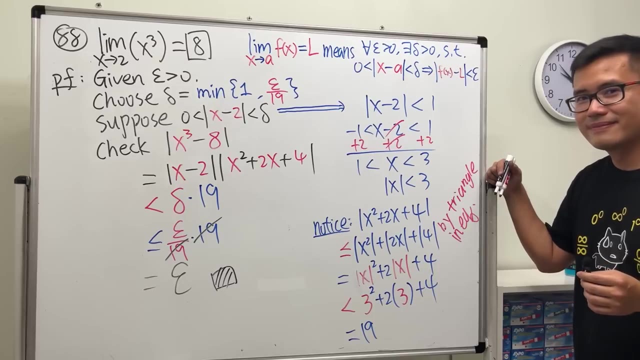 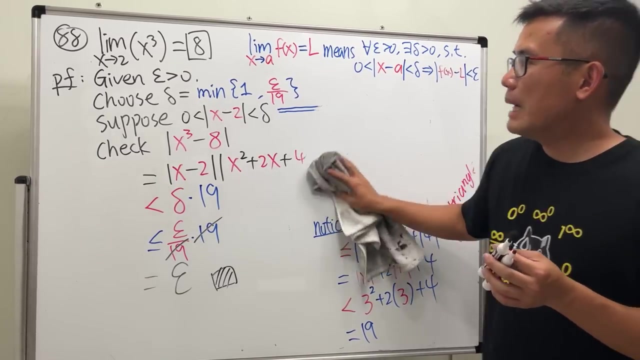 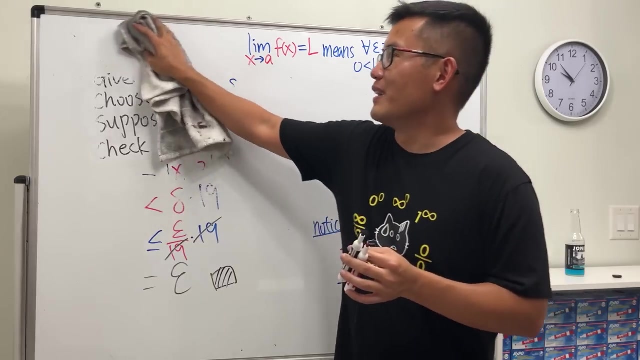 And close this Less than or equal to: Finally, don't you ever forget the box shading. What? Oh cool, Absolutely. let me have some delta definitions. A lot of fun When you know how to work it out, what you know, how to write down a good proof. 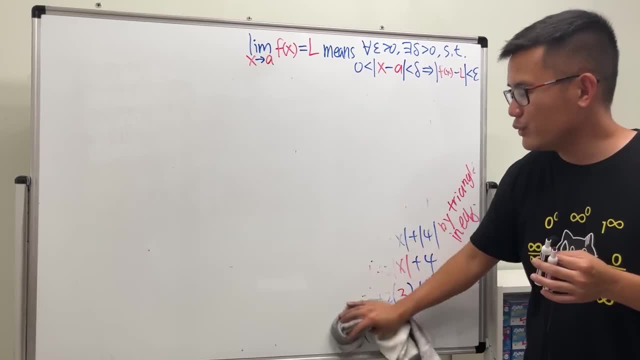 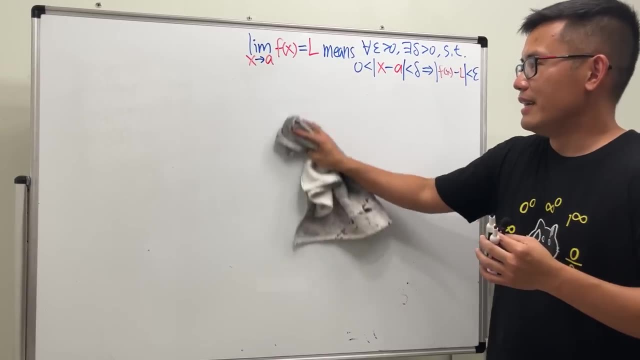 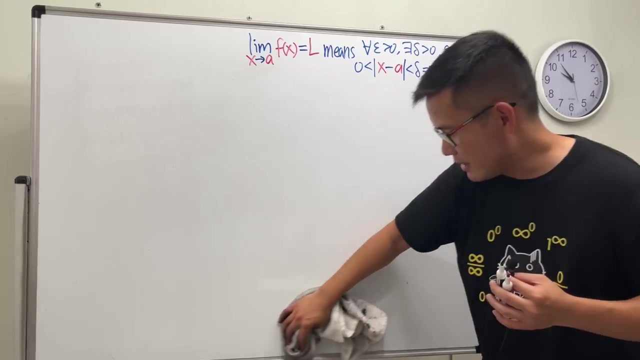 It If you. Very satisfying, very, very satisfying. yeah, I think this is the reason why a lot of people like real analysis only after they understand how to solve it, because the process of like understand it is super hard, but once you understand it, yeah the feeling. 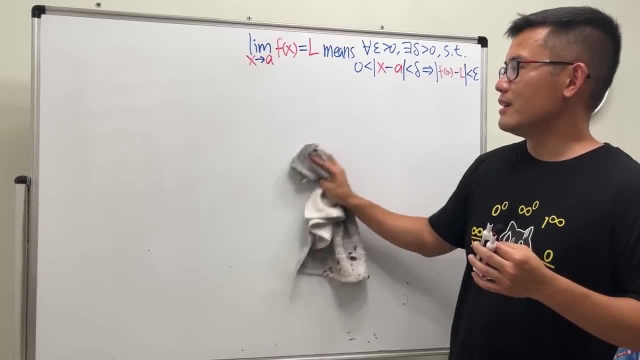 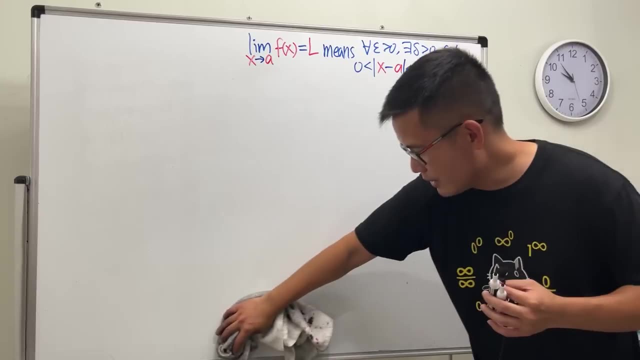 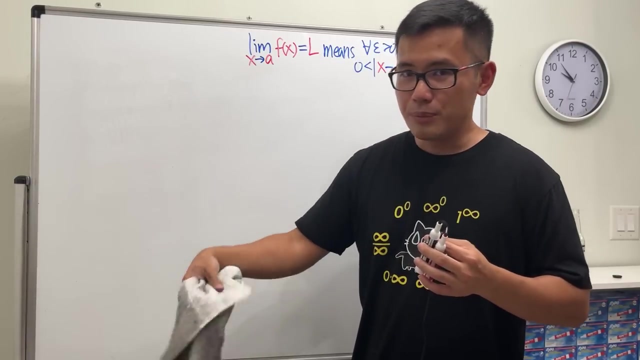 a lot of people like real analysis only after they understand how to solve it, because the process of like understanding it is super hard, but once you understand it, yeah, the feeling is super satisfying. yeah, it's like running a marathon. the running process is not that enjoyable, but after work, 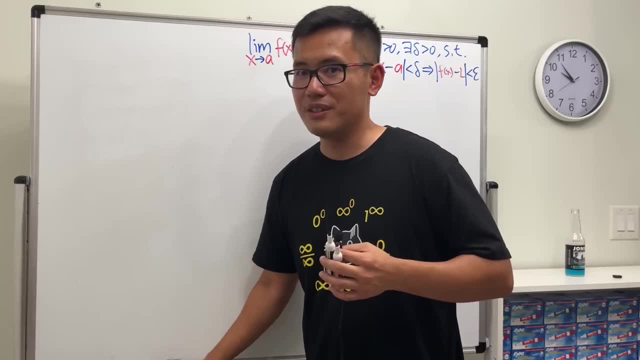 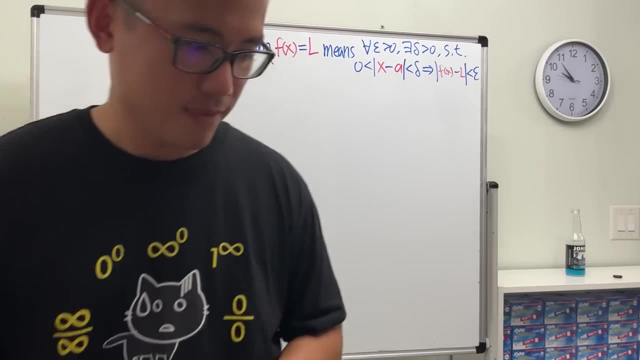 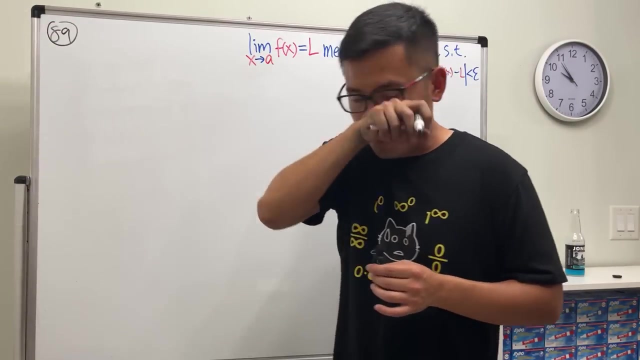 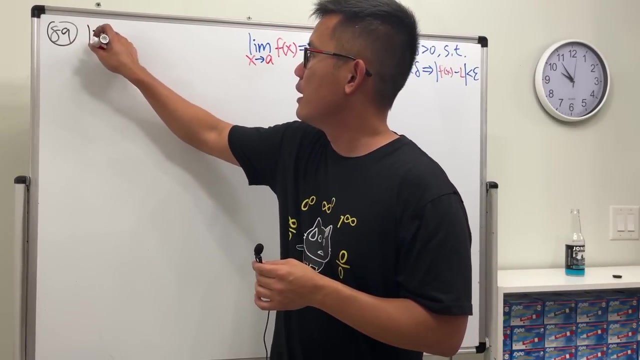 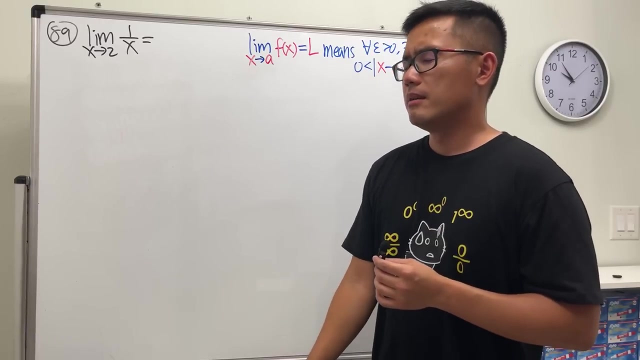 after you finish the marathon, you know it feels good, just like why I like to do 100 questions. all right. rational example number 89: all right, this is uh limit as x approaching two. yeah, this is my uh. what's that my baby calculus versus adult calculus video. 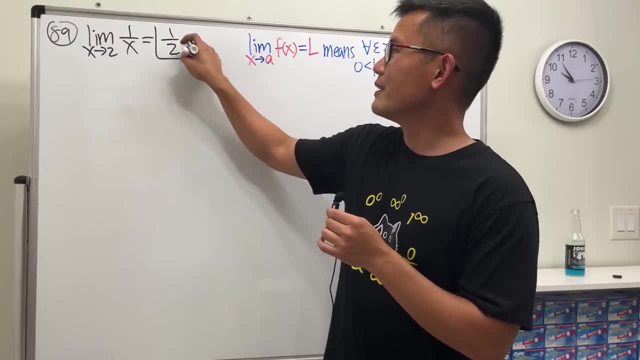 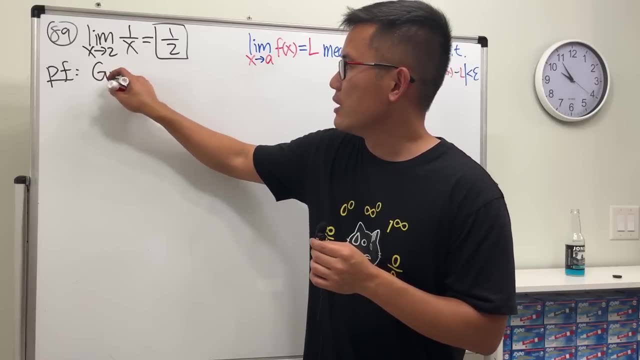 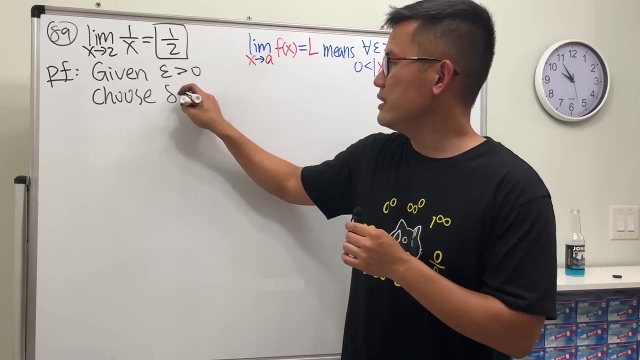 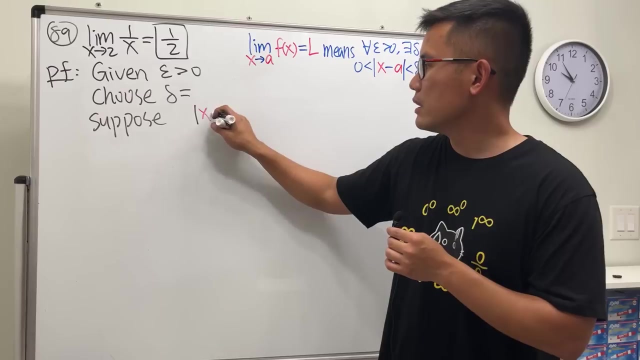 question. well, it's super easy. huh, one over two. let's take a look at the proof of it. here we go. p f, okay, given epsilon greater than zero, choose, I don't know yet. leave it. suppose we have the absolute value of x minus two is less than delta. 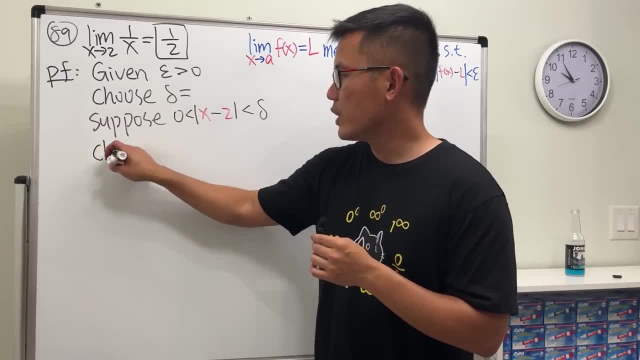 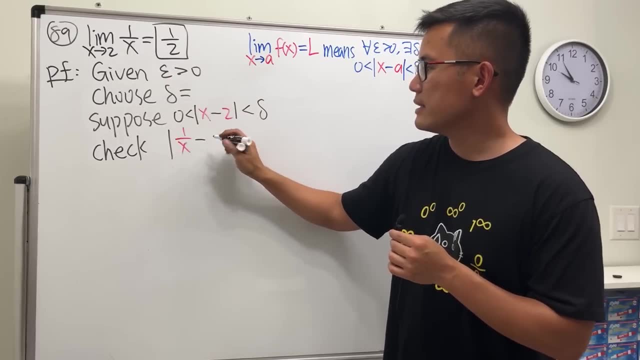 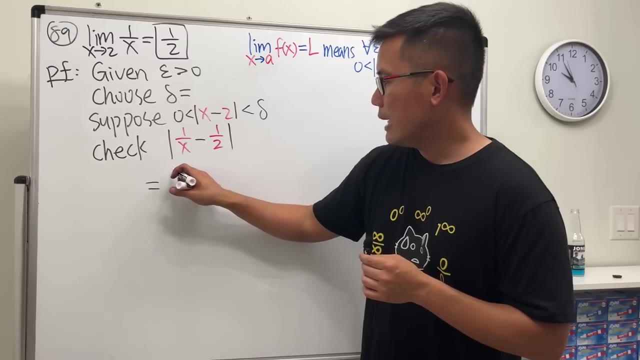 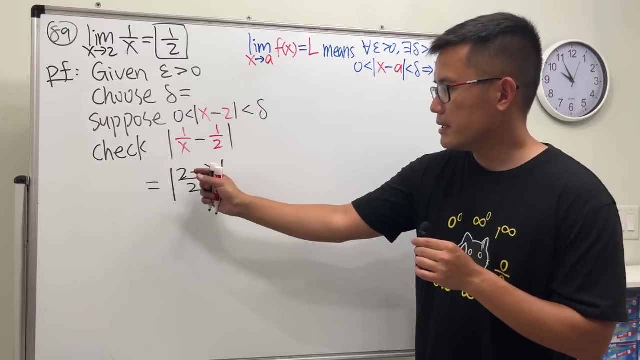 and then greater than zero, then hopefully we can get the absolute value to work for this. we want the function minus the limit. now let's do the algebra of this. get a common denominator. we get absolute value of two minus x over two x. okay, flip this subtraction so we can use that. 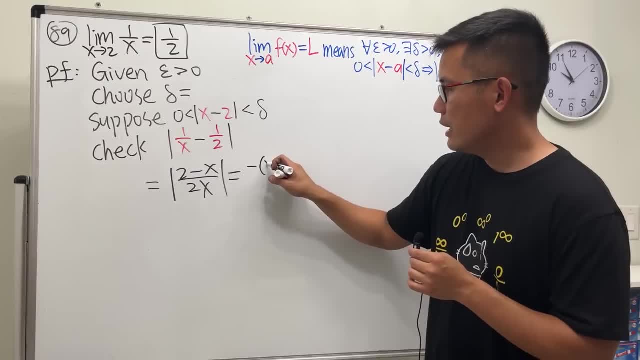 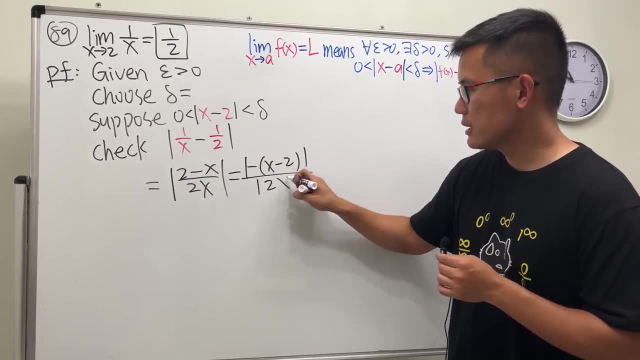 legitimately. so on the top, this right here, it's the same as negative x minus two. right, and then I can take the absolute value on the top and then the absolute value of two x. yeah, and then let's see, I'm going to write this down right here. 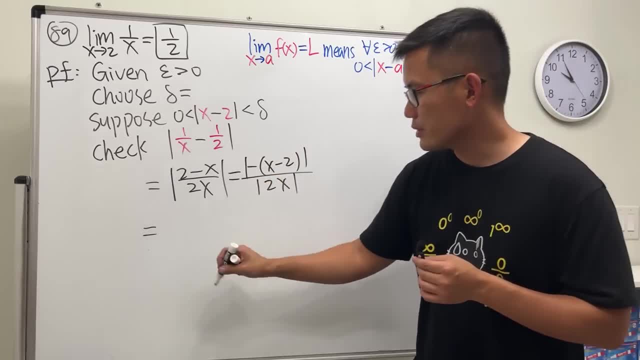 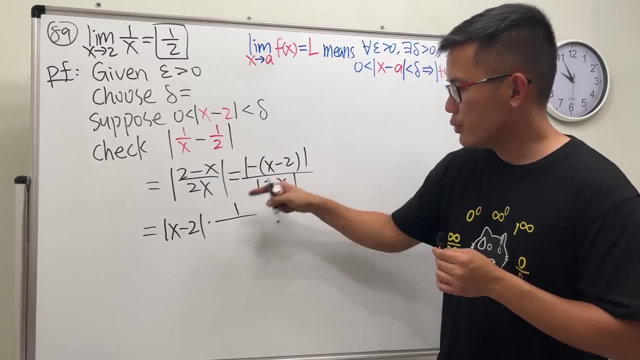 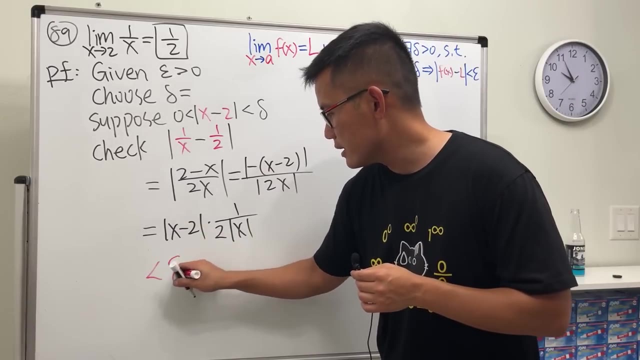 the negative in the absolute value becomes positive, so it doesn't matter. so we just have absolute value of x minus two times one over. put a two on the outside and then we have the absolute value of x. this, right here, we know, is less than delta. excellent. 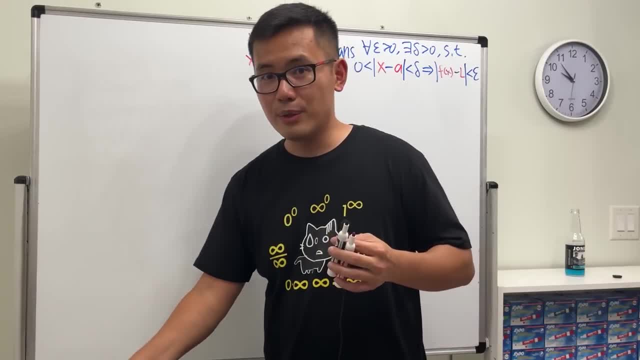 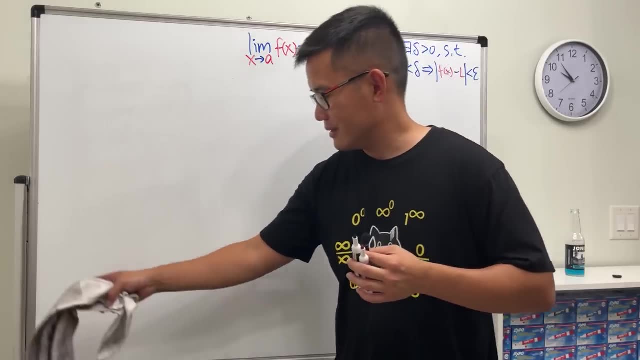 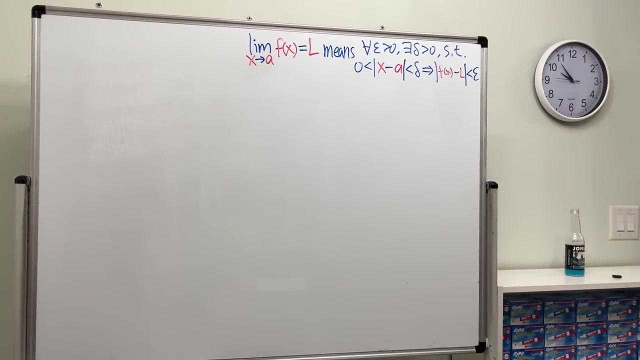 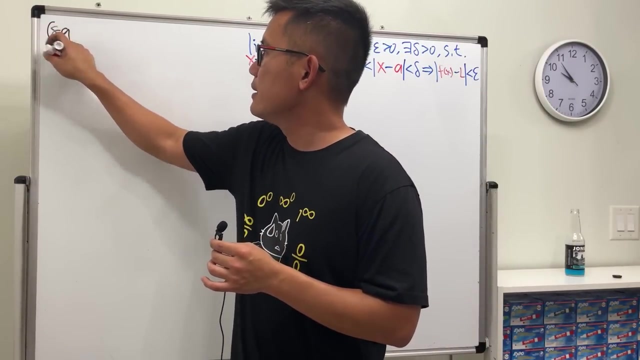 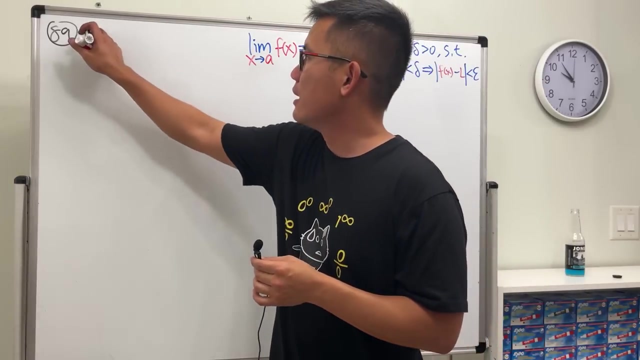 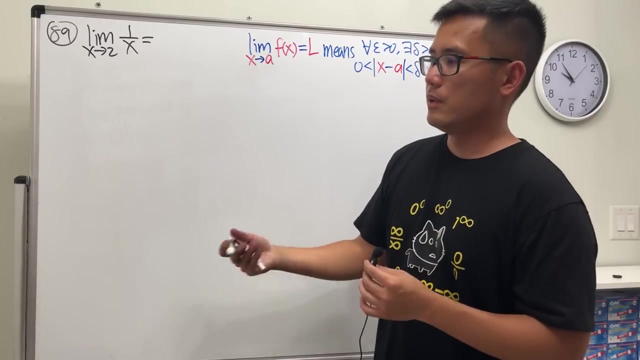 is super satisfying. yeah, it's like running a marathon. the running process is not that enjoyable, but after work, after you finish the marathon, you know feels good, just like why I like to do 100 questions. all right, rational example number 89: all right, this is a limit as X approaching to. yeah, this is my what's. that my baby calcine is going to be a baby calcine. yeah, this is my what's that. my baby calcine is going to be a baby calcine. yeah, this is my what's that. my baby calculus versus adult calculus video. calculus versus adult calculus video. 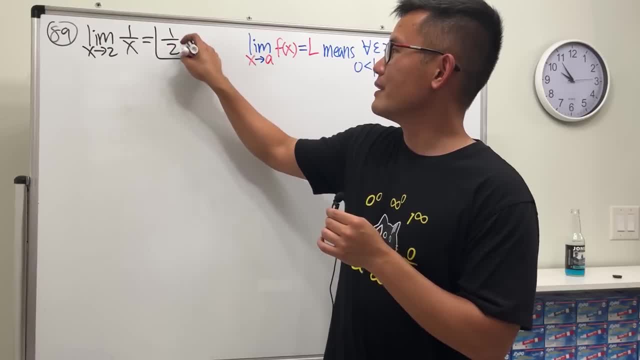 calculus versus adult calculus video question. well, it's super easy. huh 1 over question. well, it's super easy. huh 1 over question. well, it's super easy. huh, 1 over 2. let's take a look at a proof of it. 2- let's take a look at a proof of it. 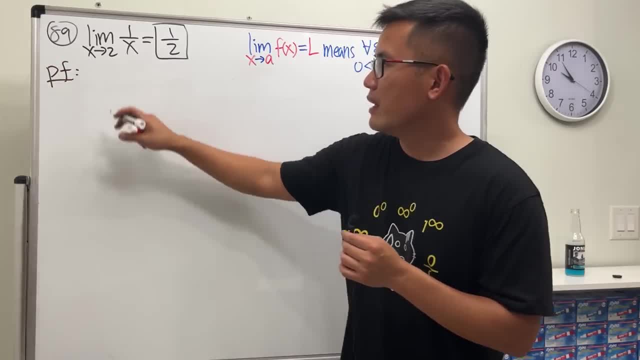 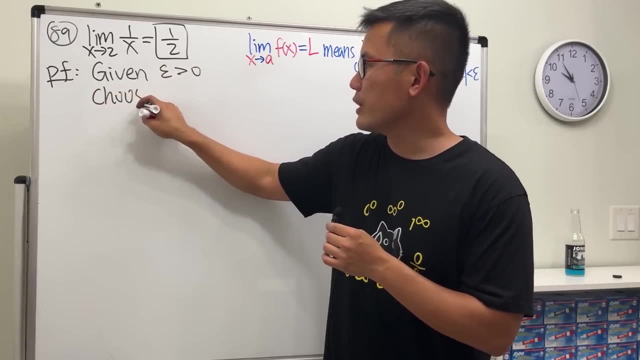 2. let's take a look at a proof of it. here we go. P F- okay, given epsilon. here we go. P F- okay, given epsilon. here we go. P F- okay, given epsilon. greater than 0- choose I don't know yet. greater than 0, choose I don't know yet. 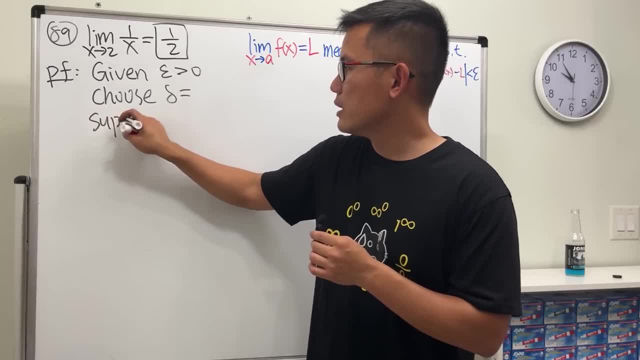 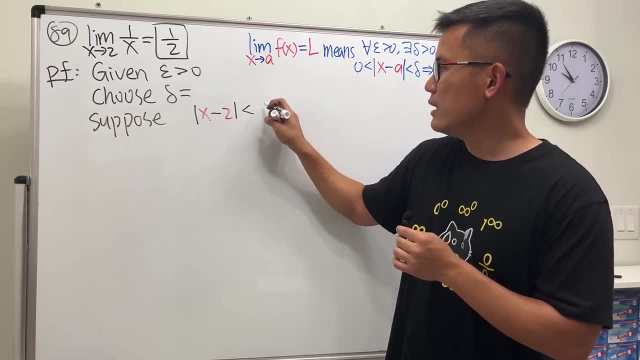 greater than 0. choose, I don't know yet, leave it. suppose we have the absolute, leave it. suppose we have the absolute leave it suppose we have the absolute value of X minus 2 is less than Delta, and value of X minus 2 is less than Delta. and 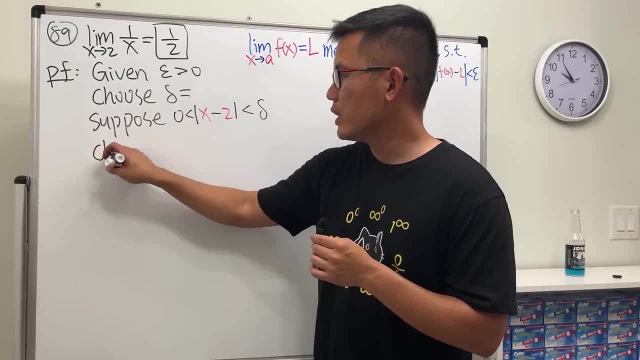 value of X minus 2 is less than Delta, and then then then greater than 0, then hopefully we can get the greater than 0, then hopefully we can get the greater than 0, then hopefully we can get the absolute value. to work for this we. 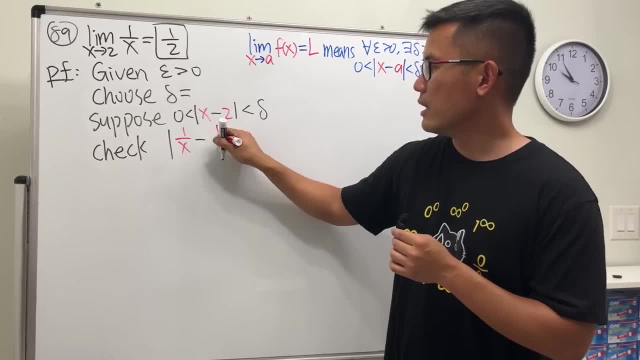 absolute value to work for this. we absolute value to work for this. we want the function minus the limit now. let's want the function minus the limit now. let's want the function minus the limit now. let's do the algebra this get a common. do the algebra this get a common. 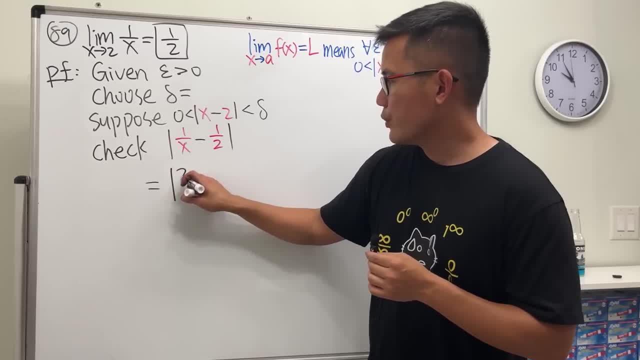 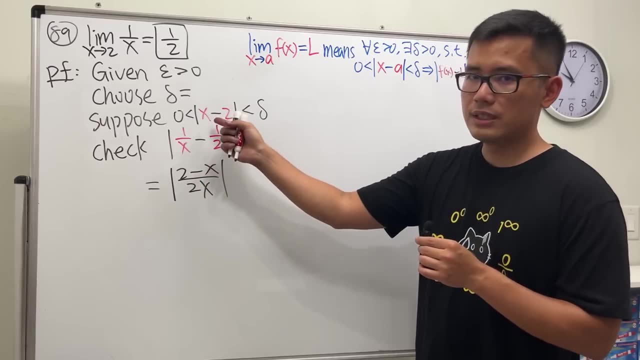 do the algebra this: get a common denominator. we get absolute value of 2 denominator. we get absolute value of 2 denominator. we get absolute value of 2 minus X over 2 X. okay, flip this minus X over 2 X. okay, flip this minus X over 2 X. okay, flip this subtraction, so we can use that. 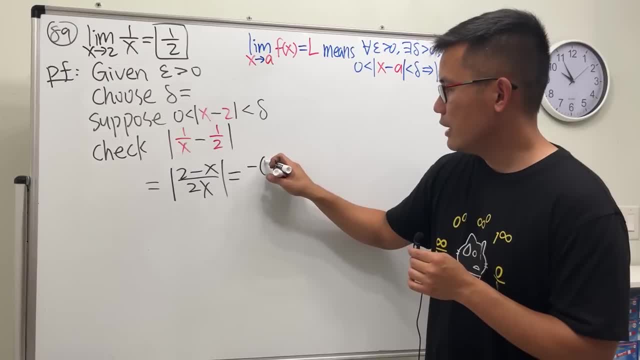 subtraction. so we can use that subtraction. so we can use that legitimately. so on the top this right legitimately. so on the top this right, legitimately. so on the top this right. here it's the same as negative X minus. here it's the same as negative X minus. 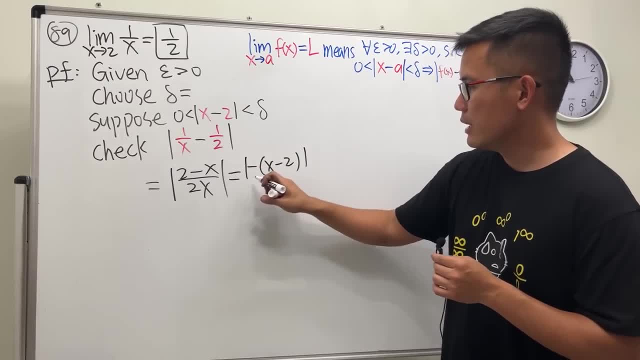 here it's the same as negative X minus 2 right, and then I can take the absolute 2 right, and then I can take the absolute 2 right, and then I can take the absolute value on the top, and then the absolute value on the top, and then the absolute. 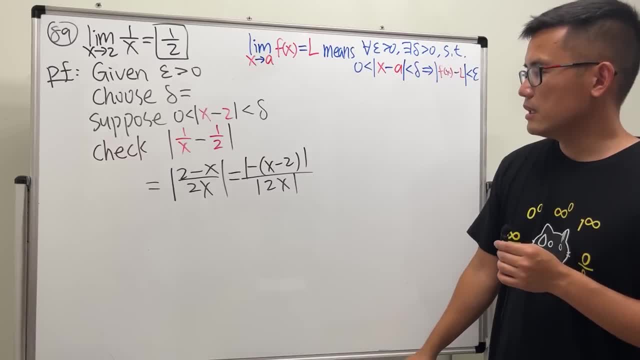 value on the top, and then the absolute value of 2x- yeah. and then let's see: I'm value of 2x- yeah. and then let's see I'm value of 2x- yeah. and then let's see- I'm going to write this down right here- the. 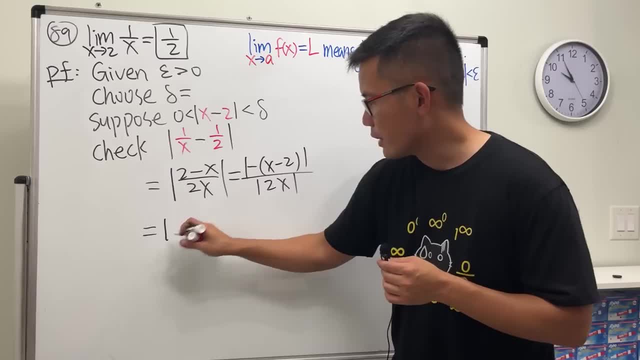 going to write this down right here. the going to write this down right here: the negative in the absolute value becomes negative in the absolute value becomes negative in the absolute value becomes positive. so it doesn't matter. so we positive. so it doesn't matter. so we positive. so it doesn't matter. so we just have absolute value of X minus 2. 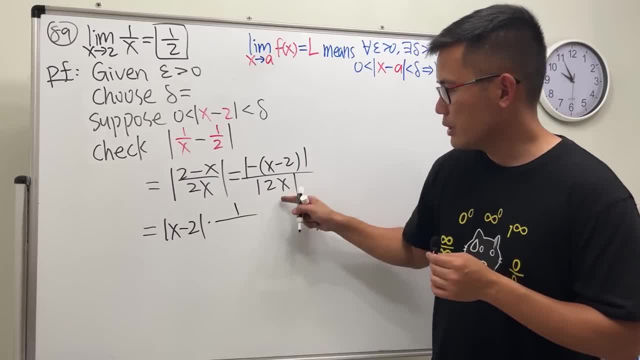 just have absolute value of X minus 2. just have absolute value of X minus 2 times 1 over. put a 2 on the outside and times 1 over. put a 2 on the outside and times 1 over. put a 2 on the outside, and then we have the absolute of X. this 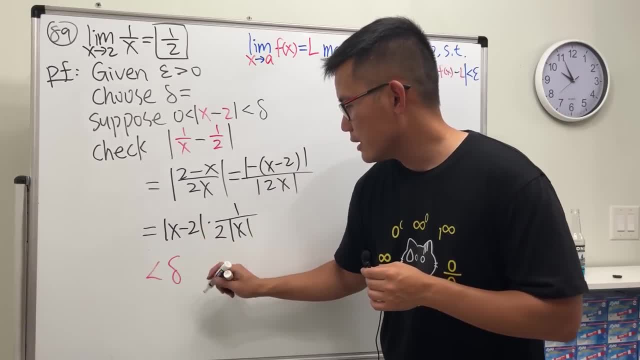 then we have the absolute of X this. then we have the absolute of X this, right here. we know it's less than Delta, right here. we know it's less than Delta. right here. we know it's less than Delta, excellent, but we don't know what this is. 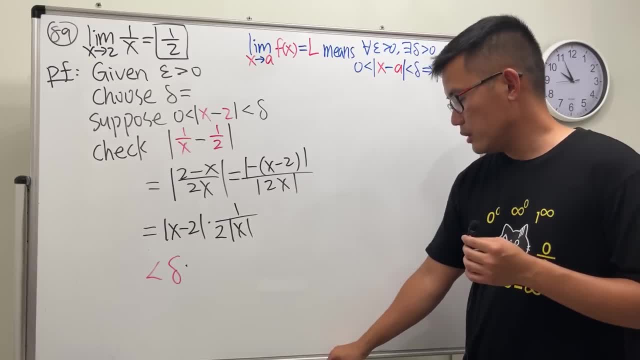 excellent, but we don't know what this is. excellent, but we don't know what this is. 1 over 2 after the 5x. so you know the 1 over 2 after the 5x. so you know the 1 over 2 after the 5x. so you know the deal. we're going to come here and say: 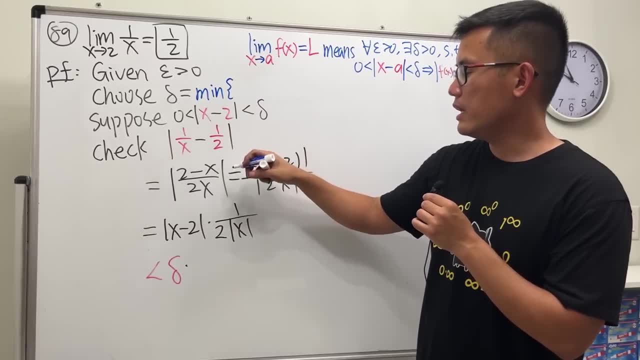 deal, we're going to come here and say, deal, we're going to come here and say Delta is equal to the minimum, and then Delta is equal to the minimum, and then Delta is equal to the minimum, and then we say 1. that way we can utilize this. 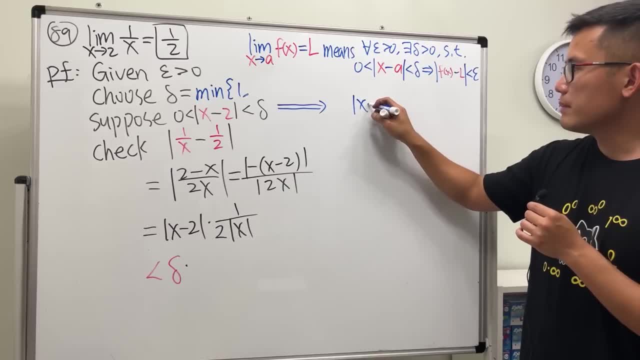 we say 1, that way we can utilize this. we say 1, that way we can utilize this. inequality, just this part after the inequality, just this part after the inequality, just this part after the failure of X minus 2 is less than 1, and failure of X minus 2 is less than 1, and 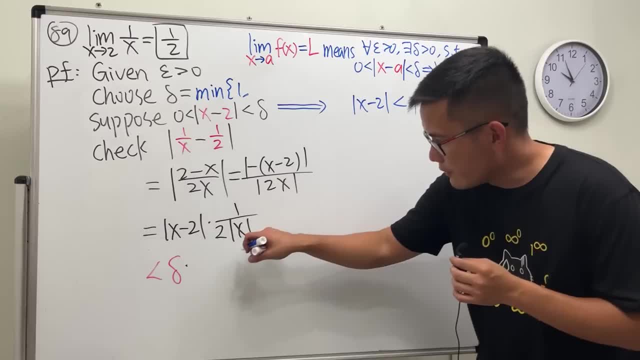 failure of X minus 2 is less than 1, and want to get this expression: huh, so want to get this expression. huh, so want to get this expression: huh. so hopefully you can find this right here. hopefully you can find this right here, hopefully you can find this right here. to be less than something, that's the 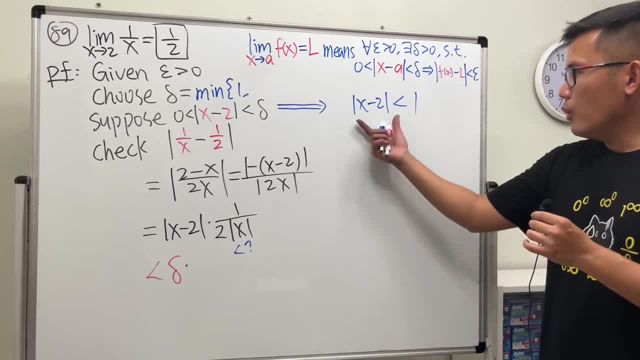 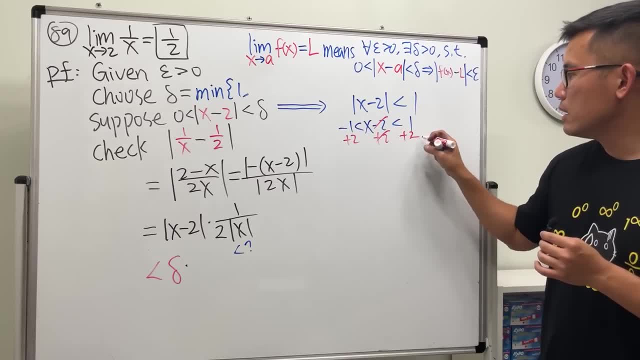 of negative 1 and 1 and then just add 2 to of negative 1 and 1, and then just add 2 to everybody we know X is in between of 1. everybody we know X is in between of 1. everybody we know X is in between of 1 and 3. this means absolute value of X is. 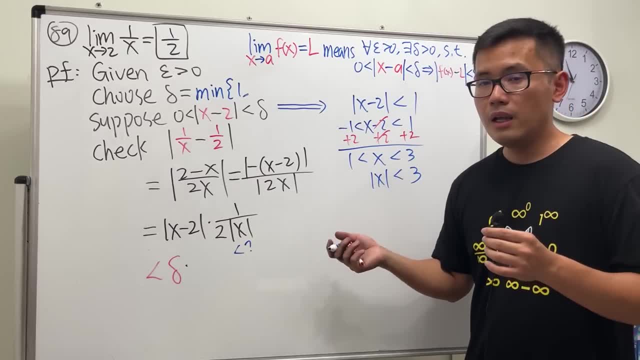 and 3. this means absolute value of X is and 3. this means absolute value of X is less than 3- right, that's what we have. less than 3- right, that's what we have. less than 3- right, that's what we have done so far, and in fact, I picked up same. 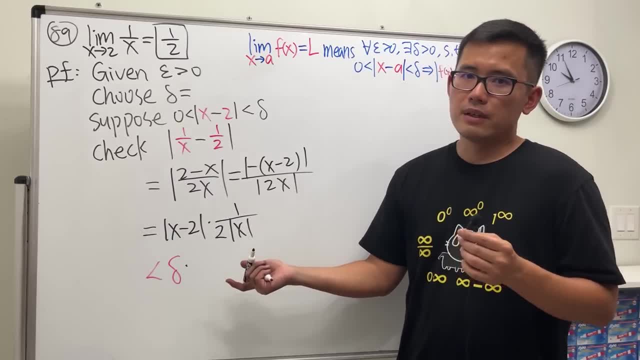 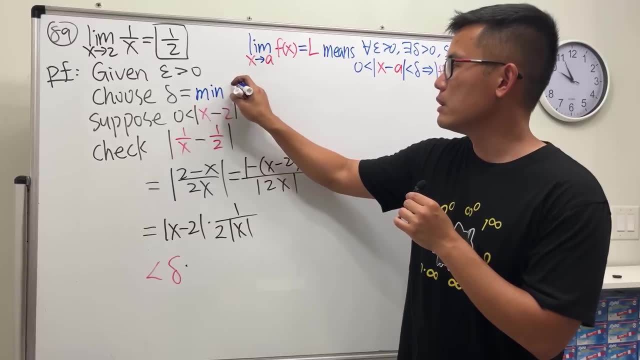 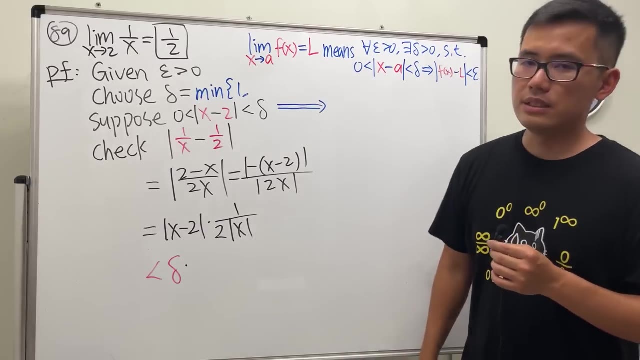 but we don't know what this is. one over two. absolute value of x. so you know the deal. we are going to come here and say delta is equal to the minimum, and then we say one. that way we can utilize this inequality, just this part. absolute value of x minus two is the. 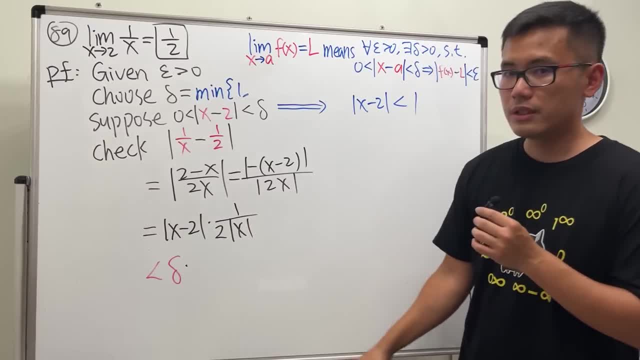 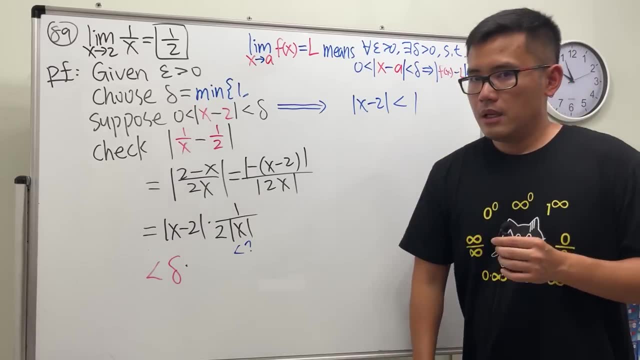 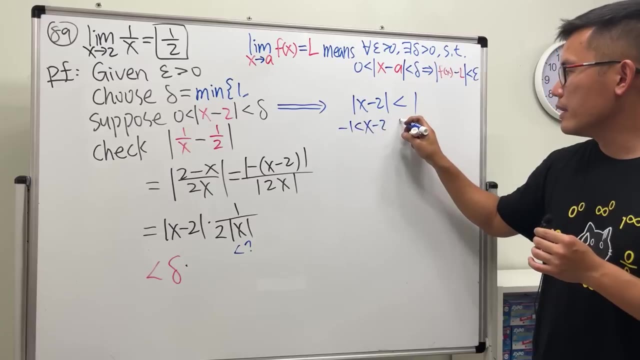 less than one and we want to get this expression- so hopefully we can find this right here- to be less than something. that's the goal. we want this to be less than something. okay, open this absolute value of x minus. this means x minus two is in between of negative one and. 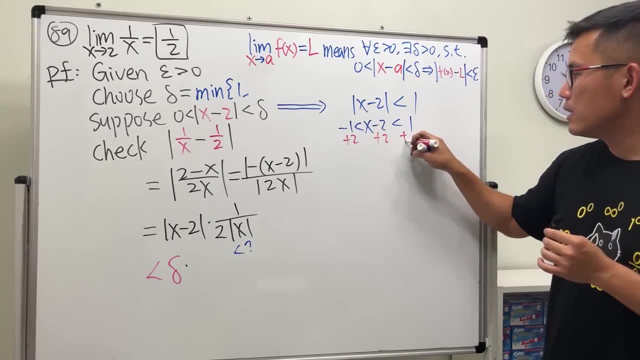 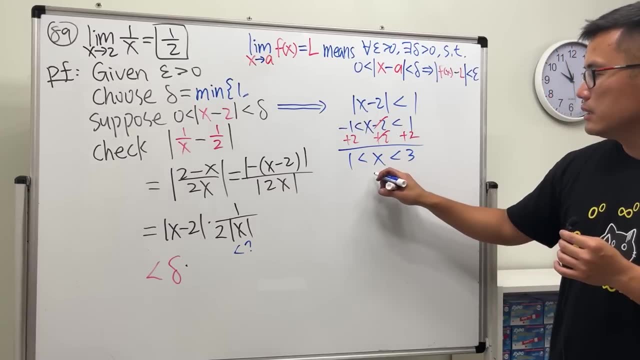 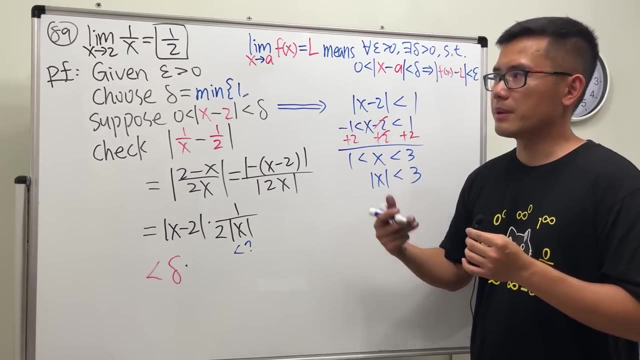 one and then just add two to everybody. we know x is in between of one and three. this means absolute value of x is less than three. right, that's what we have done so far, and in fact i picked the same number, like the previous one, on purpose. 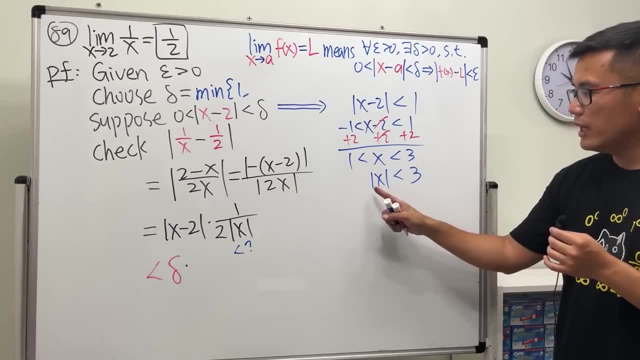 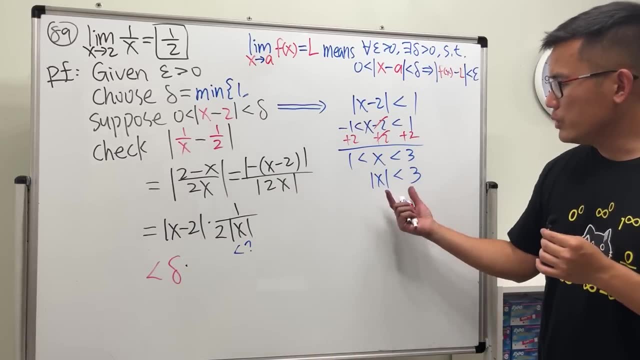 because that's what we did earlier. and now we have: absolute value of x is less than three. we want to get one over absolute value of x, so shall we just do the reciprocal right now? well, if we do that, keep in mind both sides are positive. so when we do the reciprocal, 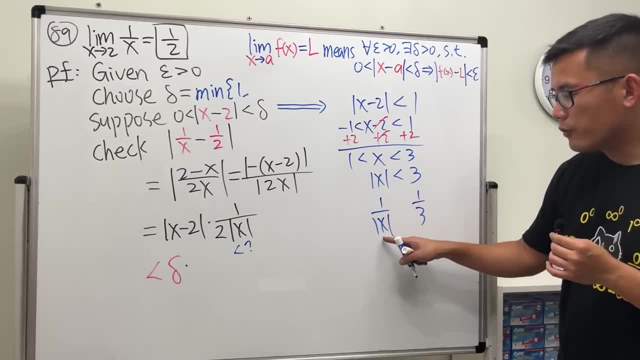 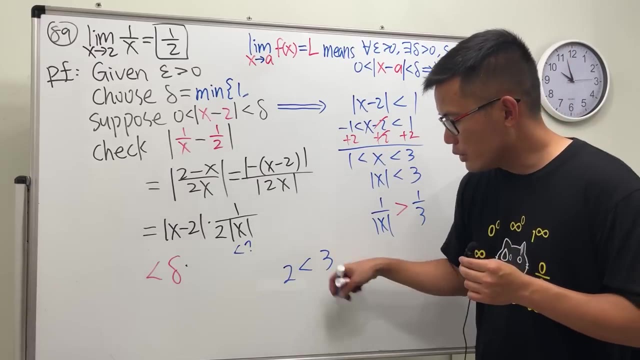 on both sides. we have one over absolute value of x and then one over three. but we will have to switch the inequality. yeah, for example, we know two is less than three, but if we do the reciprocal on both sides, in fact one half is actually bigger than one over three. 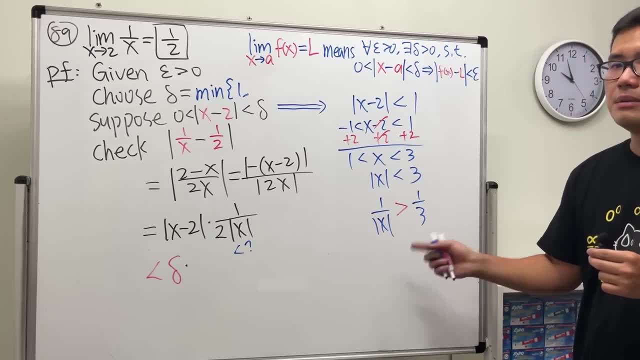 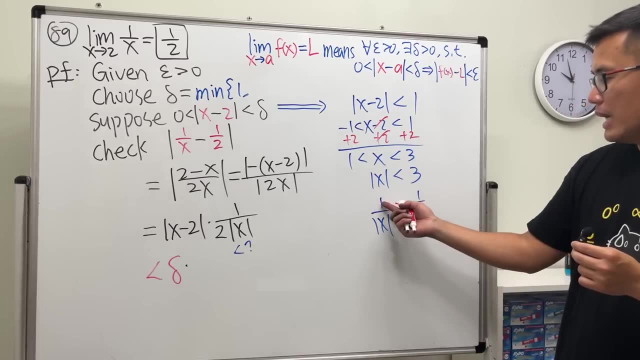 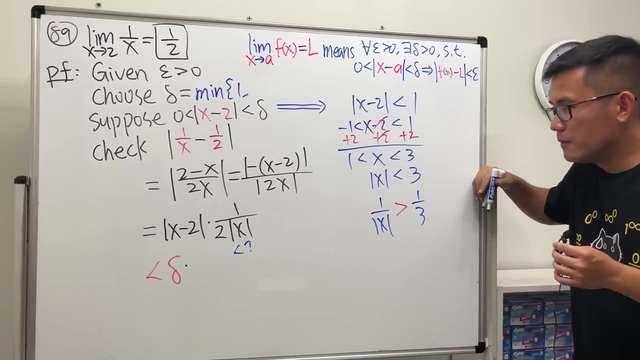 ah man, this is so bad because we cannot proceed. we really want to see this right here is less than something, but now we have one over. absolute value of x is greater than something, no good. so what do we do? i'm so stuck. no, don't worry, the trick is that. 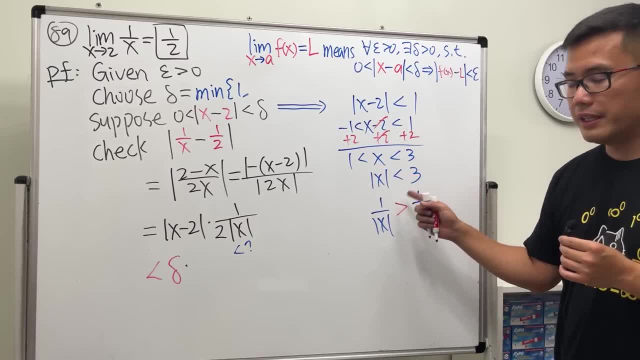 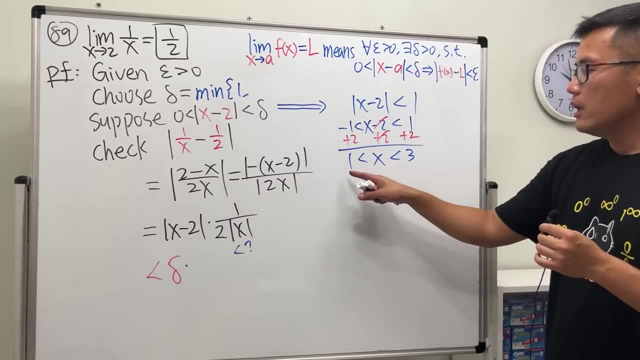 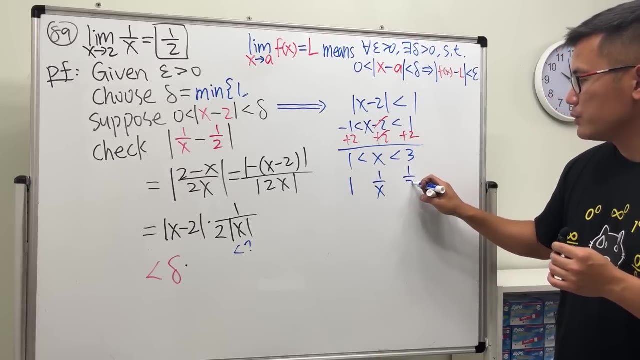 you do not do the absolute value right here, right now. in fact, we actually do the reciprocal first, and everything will go smoothly. check this out, everything is positive, so do the reciprocal. one over one is still one, and here we have one over x, and this is one over three. 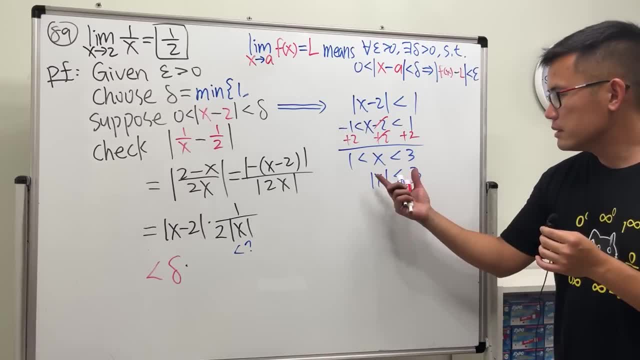 done so far and in fact I picked up same done so far and in fact I picked up same number, like the previous one on purpose number, like the previous one on purpose number, like the previous one on purpose, because that's already huh, and now we, because that's already huh, and now we. 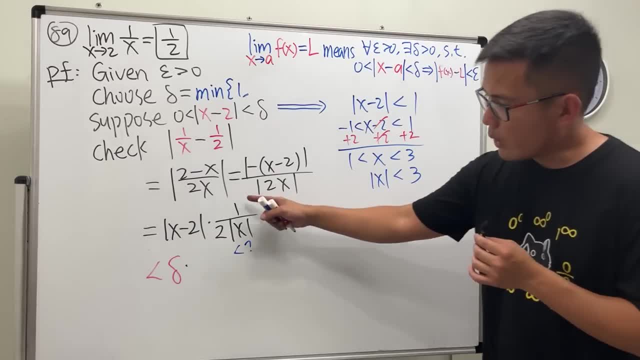 because that's already huh. and now we have: absolute value of X is less than 3. have absolute value of X is less than 3. have absolute value of X is less than 3. we want to get 1 over absolute value of. we want to get 1 over absolute value of. 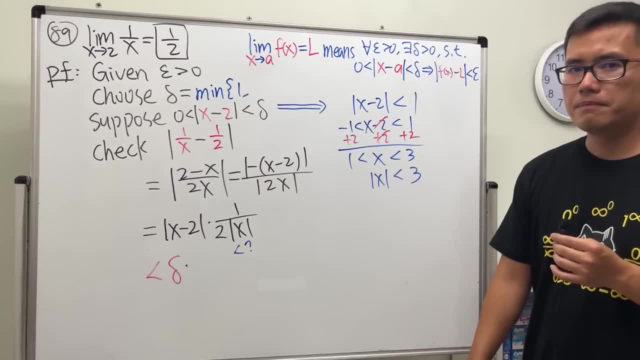 we want to get 1 over absolute value of X. so shall we just do the reciprocal X. so shall we just do the reciprocal X. so shall we just do the reciprocal right now. well, if we do that, keep in right now. well, if we do that, keep in. 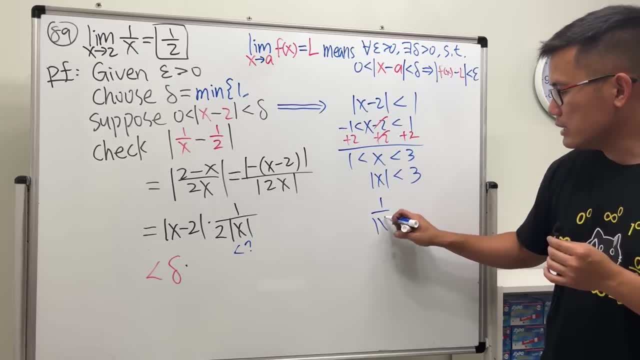 right now. well, if we do that, keep in mind, both sides are positive. so when we mind both sides are positive, so when we mind both sides are positive, so when we do the reciprocal on both sides, we have do the reciprocal on both sides, we have do the reciprocal on both sides. we have 1 over absolute value of X and then 1. 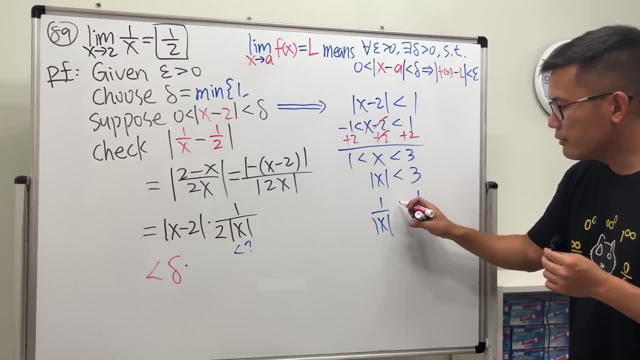 1 over absolute value of X and then 1- 1 over absolute value of X, and then 1 over 3, but we will have to switch the over 3, but we will have to switch the over 3, but we will have to switch the inequality. yeah, for example, we know 2 is. 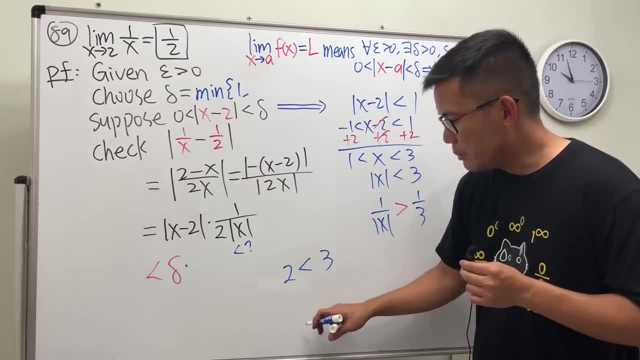 inequality. yeah, for example, we know 2 is inequality. yeah, for example, we know 2 is less than 3, but if we do the reciprocal, less than 3, but if we do the reciprocal less than 3, but if we do the reciprocal, both sides. in fact, 1 half is actually. 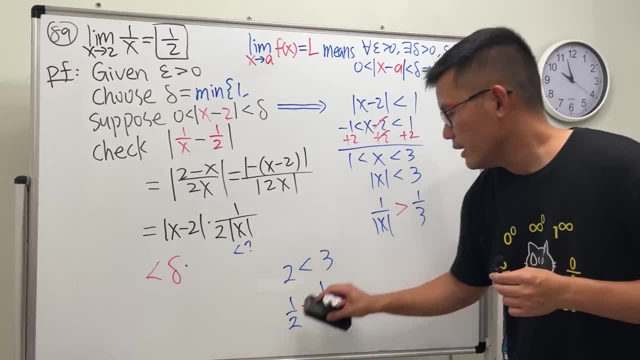 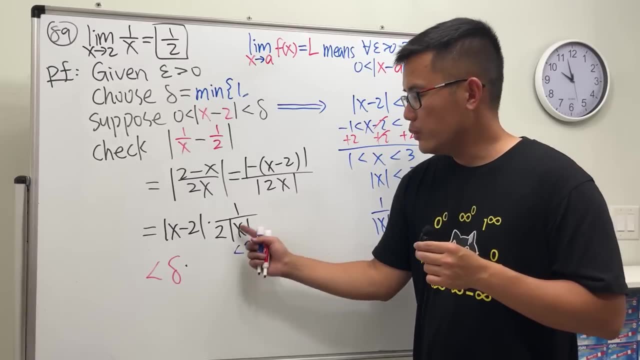 both sides. in fact, 1 half is actually both sides. in fact, 1 half is actually bigger than 1 over 3 ah man. this is so bigger than 1 over 3 ah man. this is so bigger than 1 over 3 ah man. this is so bad because we cannot proceed. we really 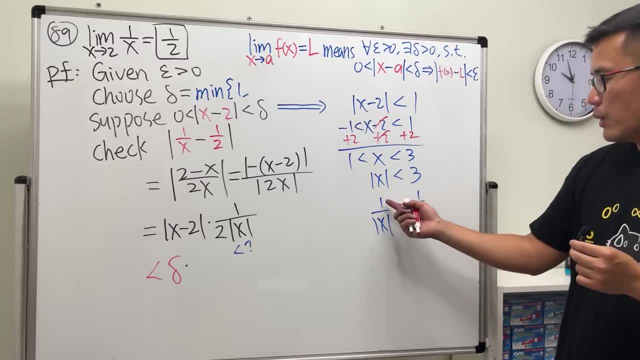 bad because we cannot proceed. we really bad because we cannot proceed. we really want to see this right here. it's less. want to see this right here, it's less. want to see this right here. it's less than something, but now we have 1 over than something, but now we have 1 over. 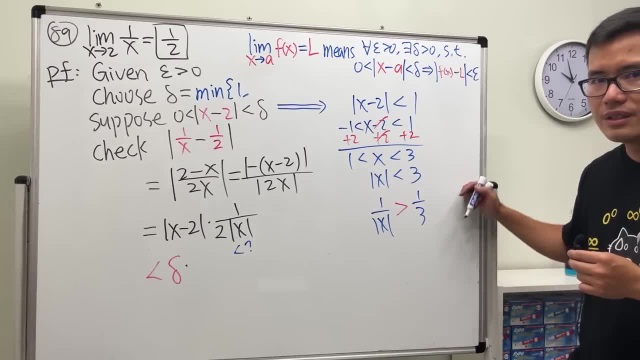 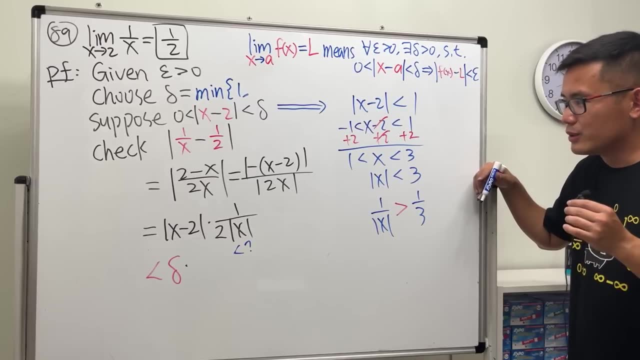 than something. but now we have 1 over. absolute value of X is greater than absolute value of X is greater than absolute value of X is greater than something no good. so what do we do? I'm something no good. so what do we do? I'm something no good. so what do we do? I'm so stuck. no, don't worry, the trick is. 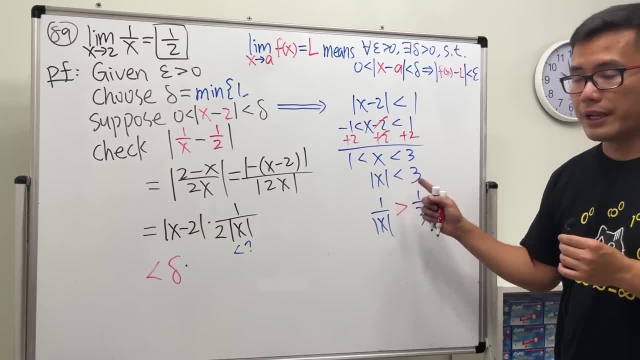 so stuck? no, don't worry, the trick is so stuck. no, don't worry. the trick is that you do not do the absolute for you, that you do not do the absolute for you, that you do not do the absolute for you right here, right now, in fact, we actually 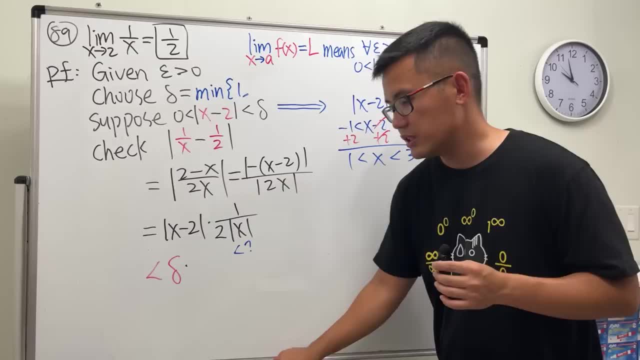 right here right now, in fact. we actually right here right now. in fact, we actually do the reciprocal first and everything. do the reciprocal first and everything. do the reciprocal first and everything will go smoothly. check this out will go smoothly. check this out will go smoothly, check this out. everything's positive. so to the 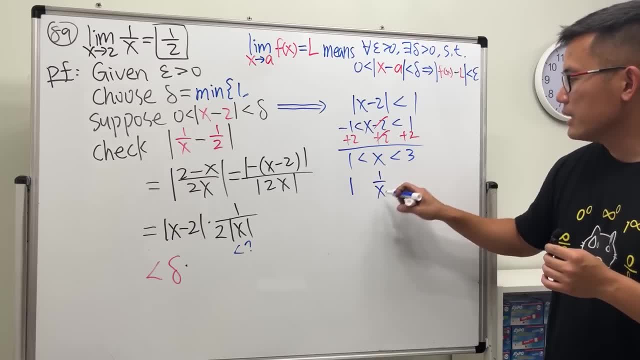 everything's positive. so to the everything's positive. so to the reciprocal: 1 over 1, still 1. and here we reciprocal 1 over 1, still 1. and here we reciprocal 1 over 1, still 1. and here we have 1 over X, and this is 1 over 3, and 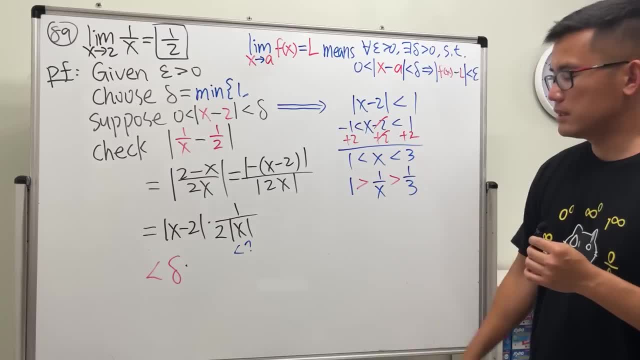 have 1 over X and this is 1 over 3, and have 1 over X and this is 1 over 3, and then flip the inequalities right this, then flip the inequalities right this, then flip the inequalities right this. this do the reciprocals first and then. 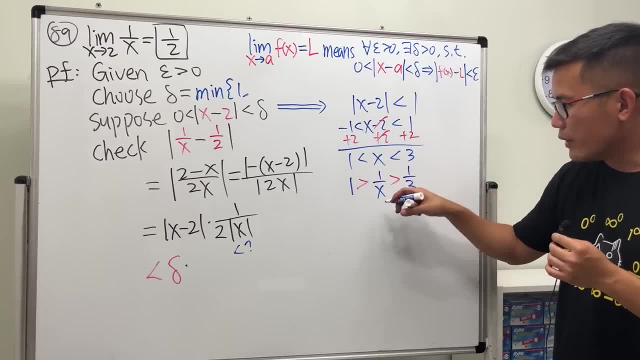 this: do the reciprocals first, and then this: do the reciprocals first, and then take the absolute value, absolute value. take the absolute value, absolute value. take the absolute value. absolute value of 1 over X is just 1 over absolute, of 1 over X is just 1 over absolute. 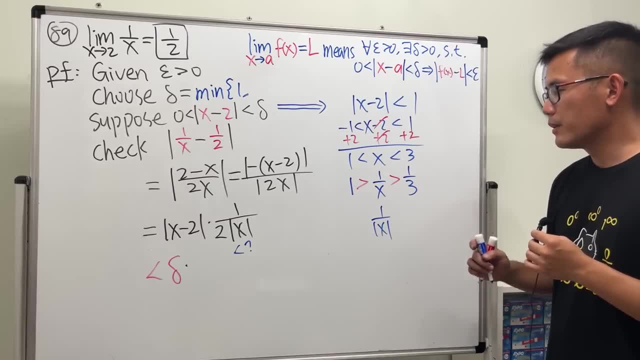 of 1 over X is just 1 over absolute x. that should be clear. and now which one x? that should be clear. and now which one x. that should be clear. and now which one. has a big absolute value 1, so in fact has a big absolute value 1, so in fact. 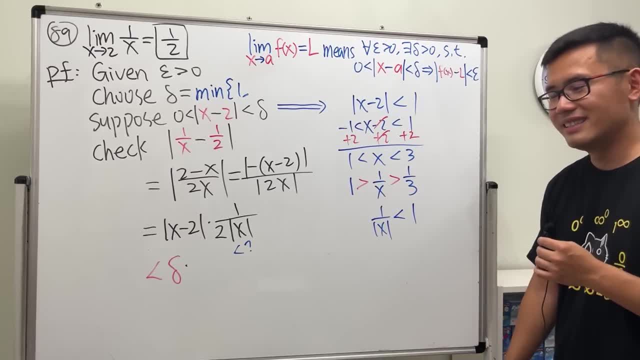 has a big absolute value: 1. so in fact, this right here is less than 1, and then this right here is less than 1, and then this right here is less than 1, and then minus will put a 2 right. yes, well as minus will put a 2 right. yes, well as. 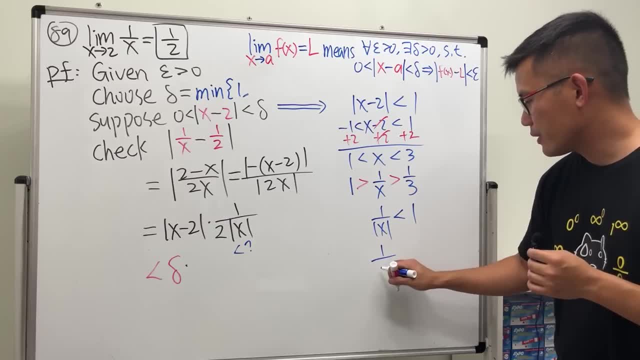 minus will put a 2 right. yes, well, as it's 2 on the bottom, though. so let's it's 2 on the bottom, though. so let's it's 2 on the bottom, though. so let's multiply both sides by 2, so 1 over 2. 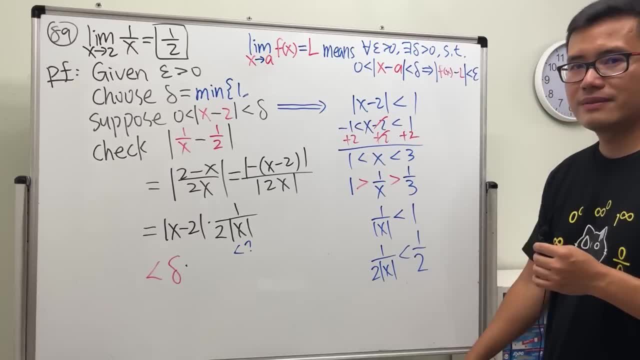 multiply both sides by 2, so 1 over 2. multiply both sides by 2, so 1 over 2. absolute of X. this right, yes, that's the absolute of X. this right, yes, that's the absolute of X. this right, yes, that's the one half this, and we have the less than. 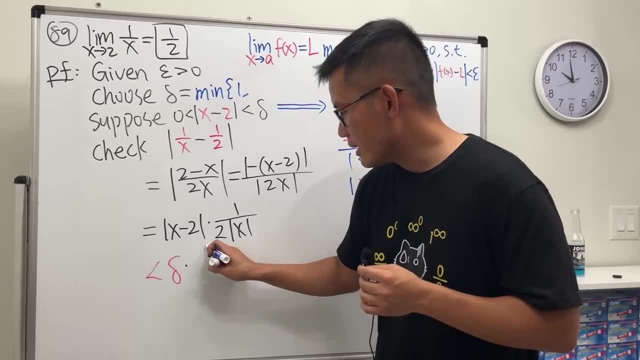 one half this, and we have the less than one half this and we have the less than already very good. we know this right already very good. we know this right already very good. we know this right: here is dense down one half, so what do. here is dense down one half, so what do? 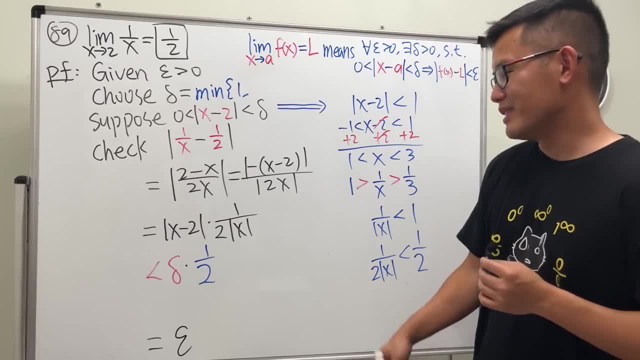 here is dense down one half. so what do we need for the Delta? this one is we need for the Delta. this one is we need for the Delta. this one is rather special. huh, we want to tell her rather special. huh, we want to tell her rather special. huh, we want to tell her to be 2 epsilon. because this way, when we 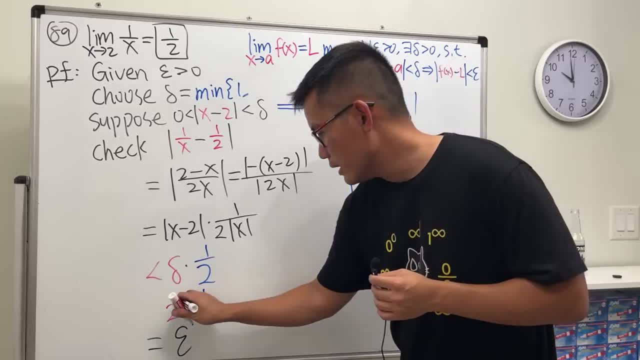 to be 2 epsilon. because this way, when we to be 2 epsilon. because this way, when we multiply by 1 over 2, the 2 and 2 will multiply by 1 over 2, the 2 and 2 will multiply by 1 over 2, the 2 and 2 will cancel. so hurry up, let's put out how to. 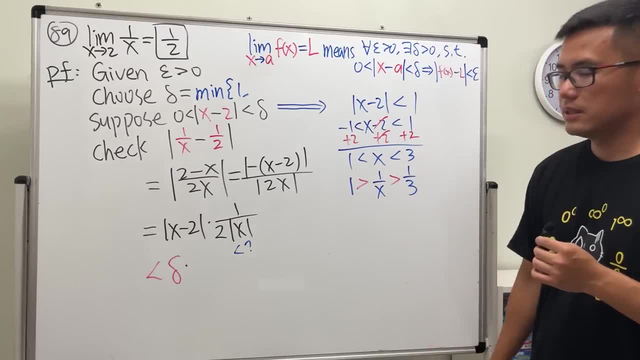 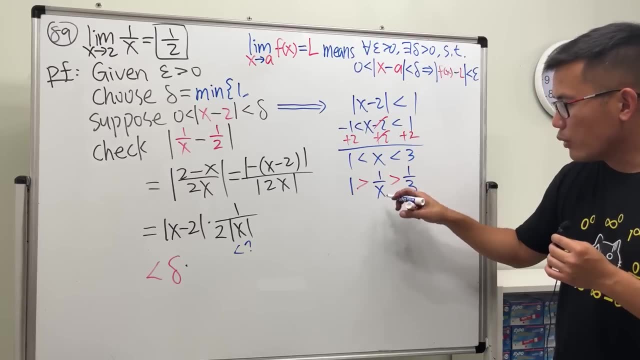 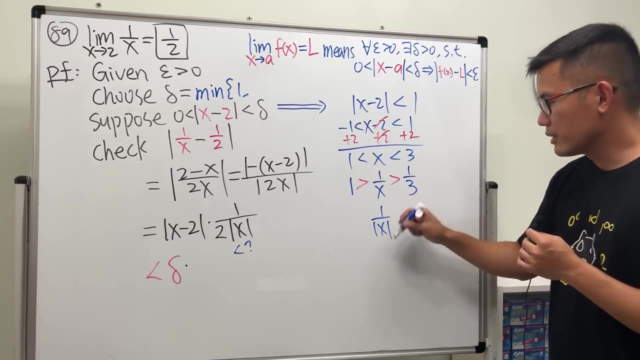 and then flip the inequalities right. this, this, do the reciprocals first and then take the absolute value. absolute value of one over x is just one over absolute value of x. that should be clear. and now, which one has a bigger absolute value? one. so in fact this: 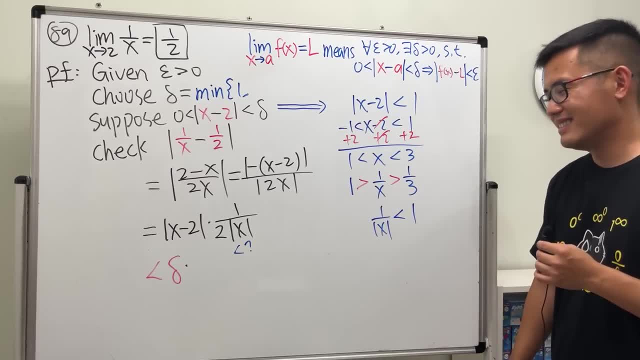 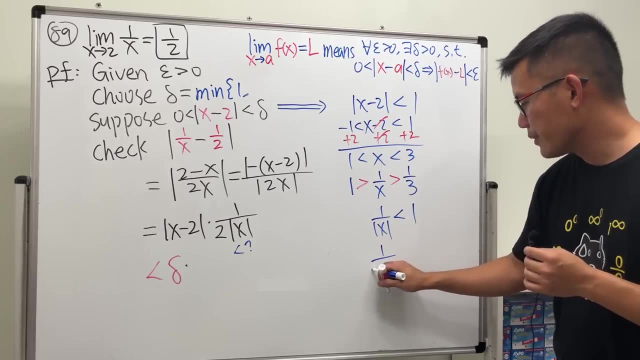 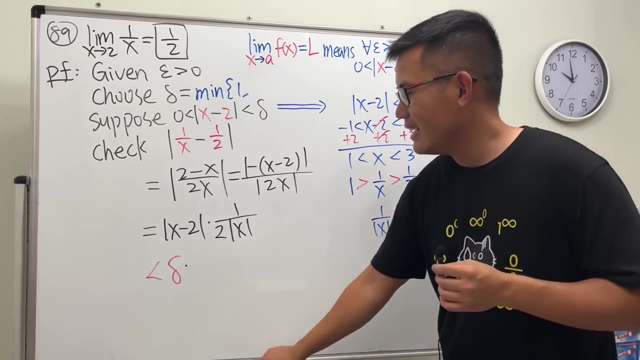 right here is less than one. yeah, and then minus. we will put a two right here as well as two on the bottom, though, so let's multiply both sides by two, so one over two. absolute value of x. this right here is less than one, half this, and we have the less than already. 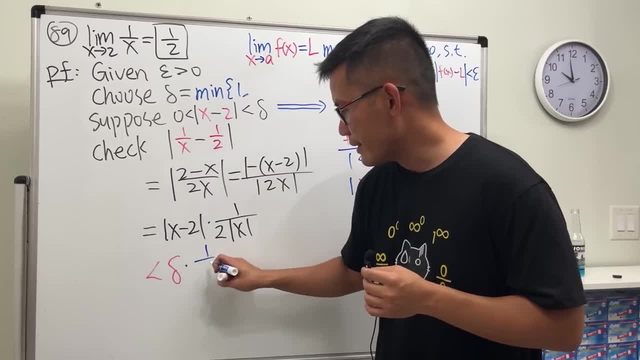 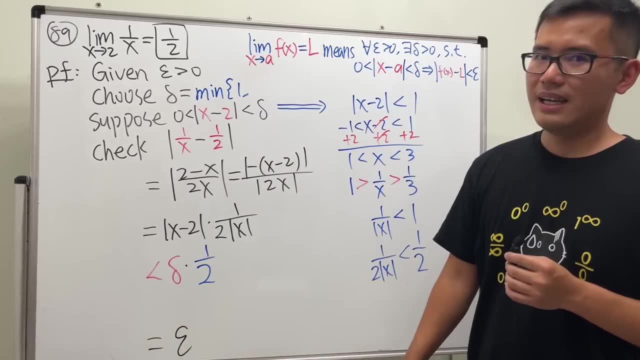 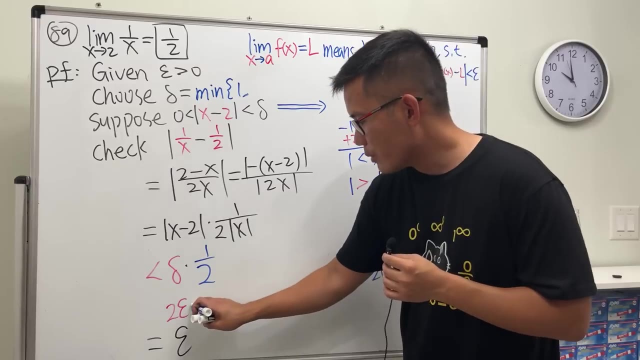 very good, we know this right here is less than one half. so what do we need for the delta? this one is rather special, huh, we want the delta to be two epsilon, because this way, when we multiply by one over two, the two and two will cancel. so so hurry up. 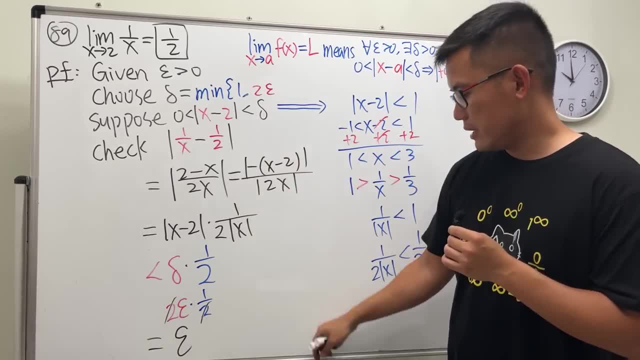 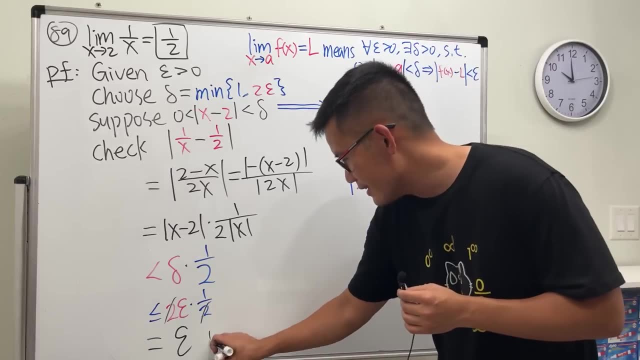 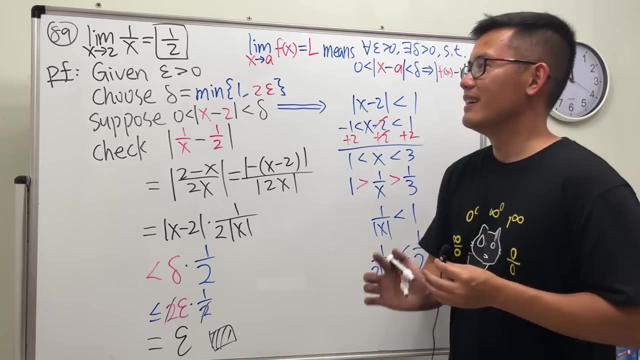 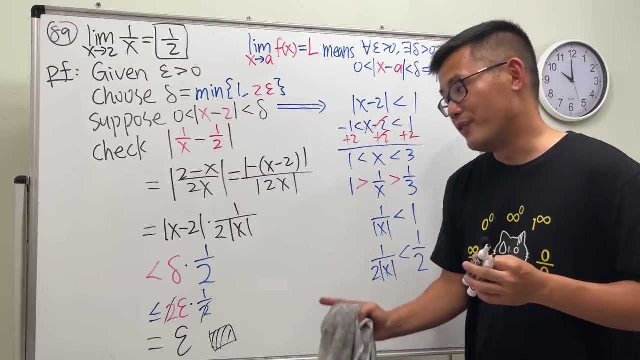 let's put delta to be two epsilon here and then close this and then it's a minimum, so and then finally draw the box, shake this in. yeah, hey, if you feel good with epsilon delta definition, don't worry, there's one more. and for the last one i'm 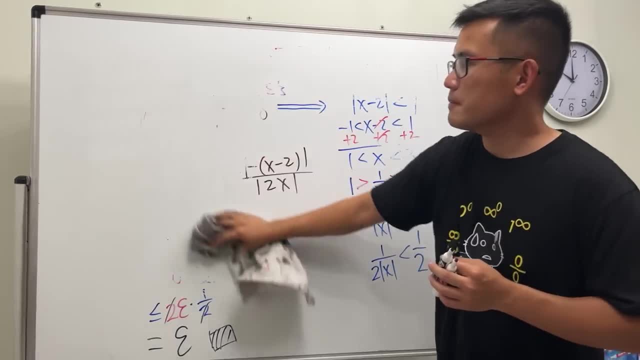 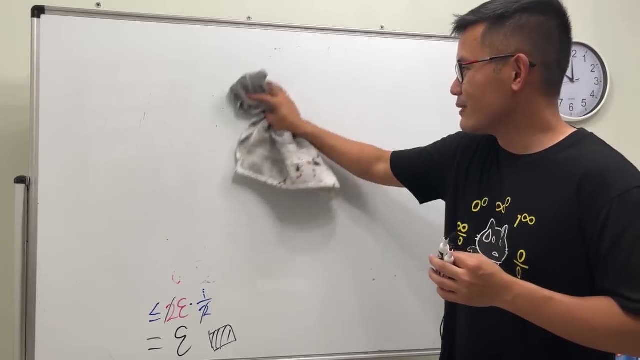 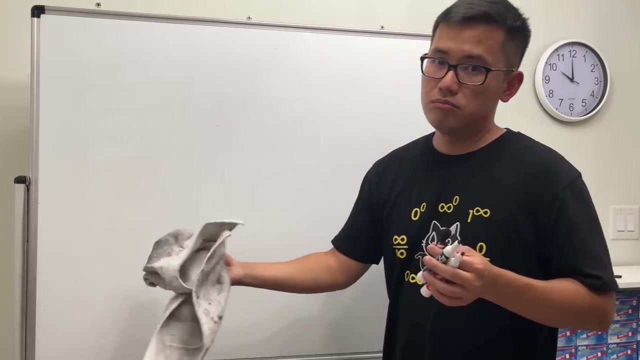 going to erase that as well, right, so i'm going to see if we can record everything. i think we have been doing a good job recording all the definitions, right, all the steps. so you see, after tenth epsilon delta definition in a row, it's not so bad, huh. 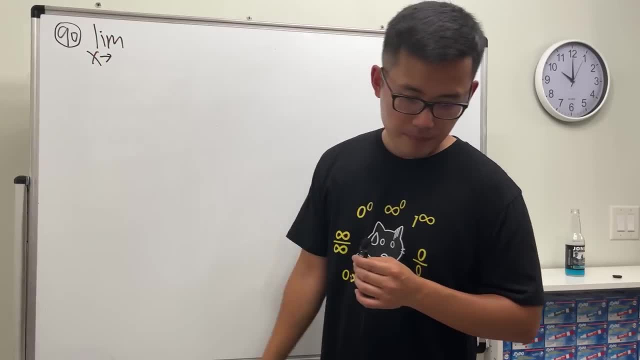 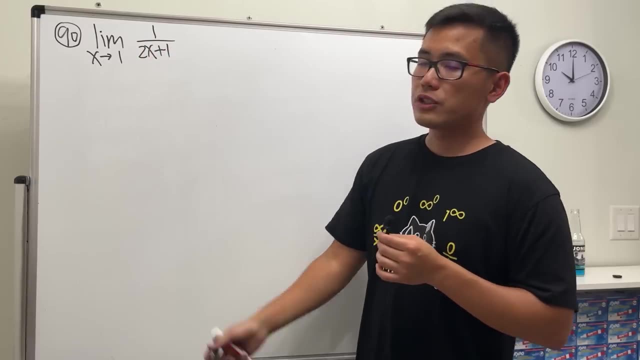 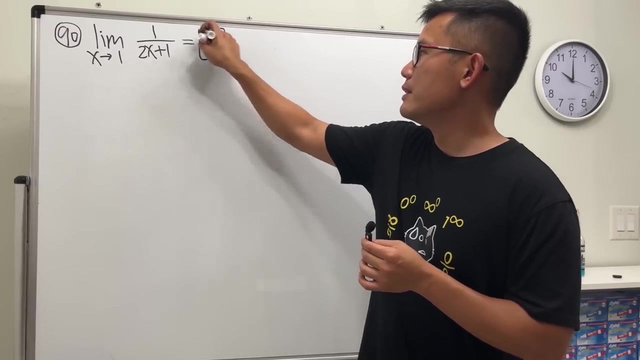 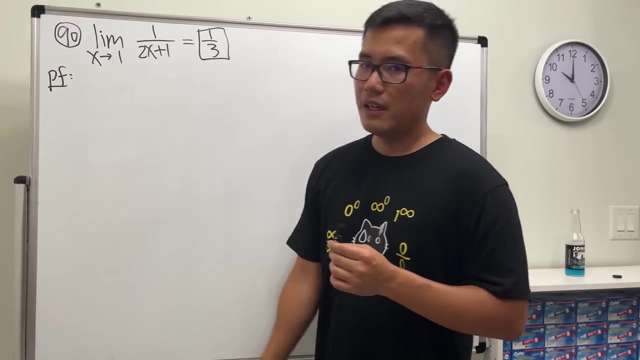 right limit as x approaching one. as i said, another rational case, and for this one put one in. there worked out like one third. so simple, but yet it's going to be also pretty difficult. don't worry, though, i'll take care of you guys. pf: first given. 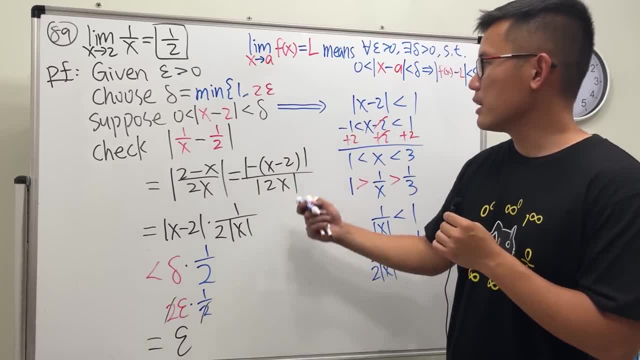 cancel. so hurry up, let's put out how to cancel. so, hurry up, let's put out how to be 2 epsilon here and then close this. be 2 epsilon here and then close this. be 2 epsilon here and then close this, and then it's a minimum, so true, and then 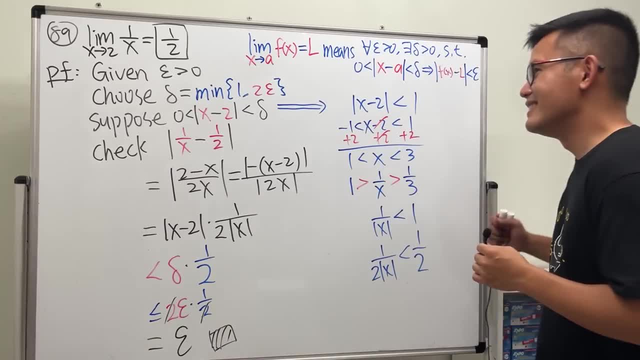 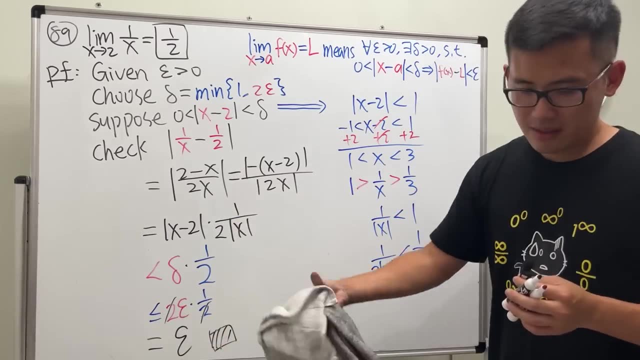 and then it's a minimum, so true. and then, and then it's a minimum, so true. and then, finally draw the box, say the same. finally draw the box, say the same. finally draw the box, say the same. yeah, hey, if you feel good with Epson Delta. 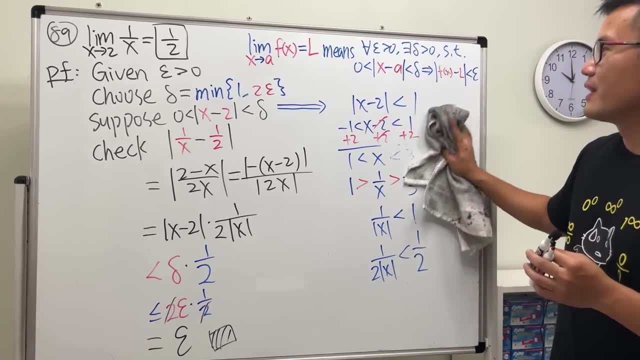 hey, if you feel good with Epson Delta, hey, if you feel good with Epson Delta. definition- don't worry this one more. and definition- don't worry this one more. and definition- don't worry this one more. and for the last one, I'm going to erase that. 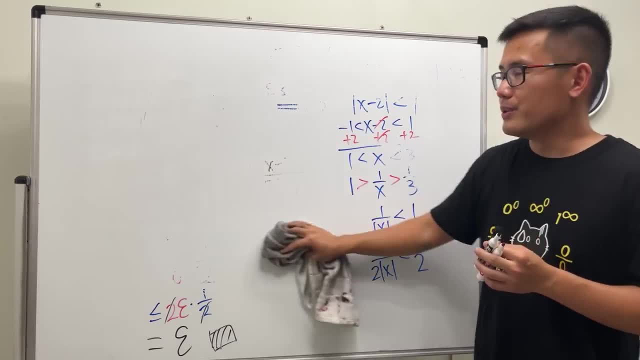 for the last one. I'm going to erase that. for the last one. I'm going to erase that as well. right? so I'm going to see if we as well, right? so I'm going to see if we as well, right? so I'm going to see if we can recall everything I think we have. 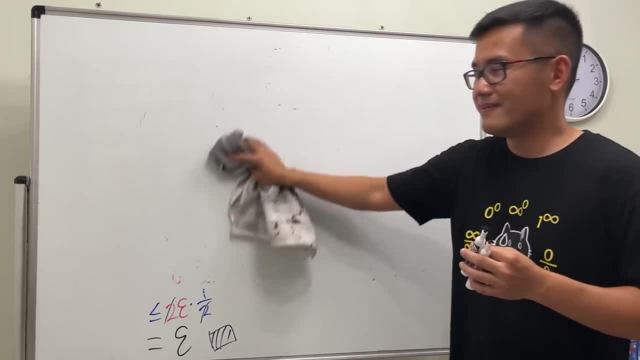 can recall everything I think we have, can recall everything I think we have been doing a good job, recording all the been doing a good job, recording all the been doing a good job, recording all the definitions right, all the steps so you. definitions right, all the steps so you. 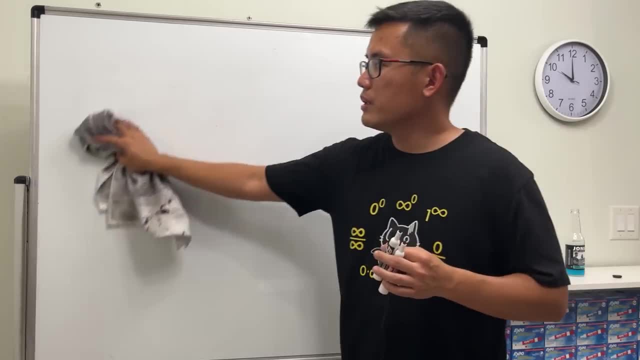 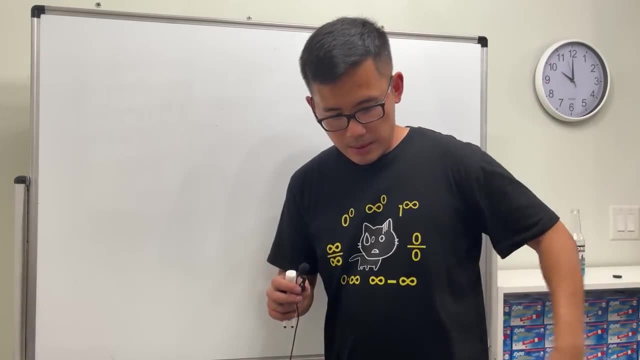 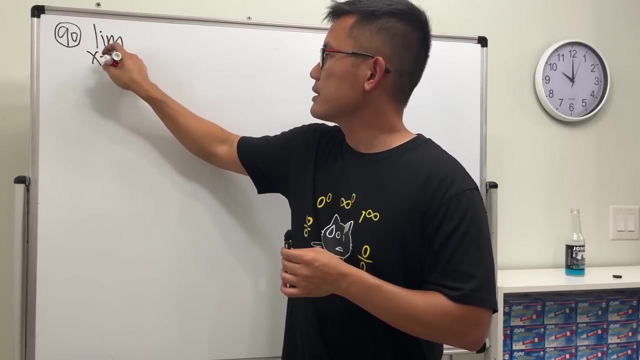 definitions. right, all the steps. so you see after 10 Epson Delta definition in see. after 10 Epson Delta definition in see after 10 Epson Delta definition in a row. it's not so better. right limit has X approaching one as I. right limit has X approaching one as I. 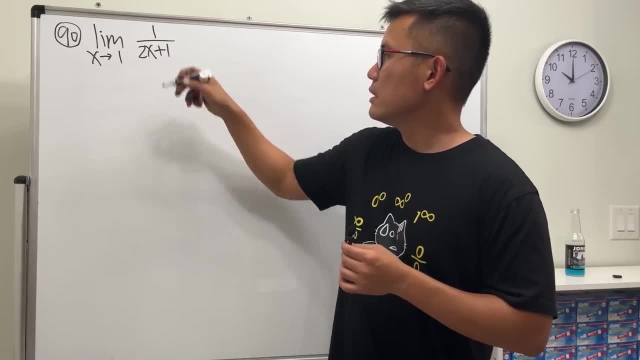 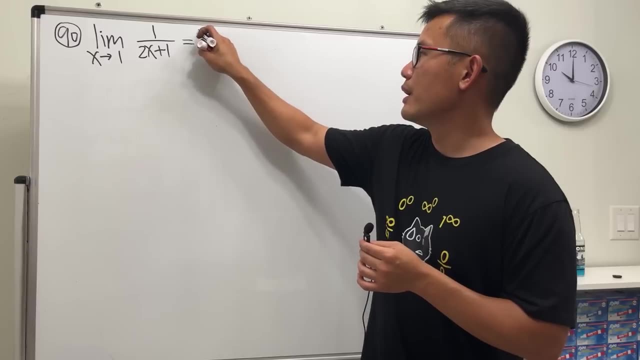 right limit has X approaching one. as I said, another rational case. and for this said another rational case. and for this said another rational case. and for this: one put one in there, worked out. we one put one in there, worked out. we one put one in there, worked out. we could one third. so simple, but yet it's. 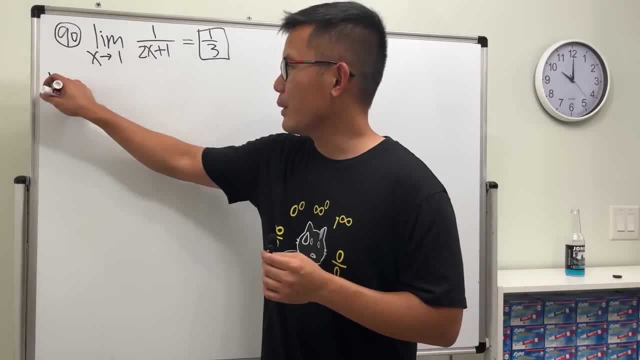 could one third so simple, but yet it's could one third so simple, but yet it's going to be also pretty difficult. don't going to be also pretty difficult? don't going to be also pretty difficult. don't worry, though, I'll take up you guys PF. 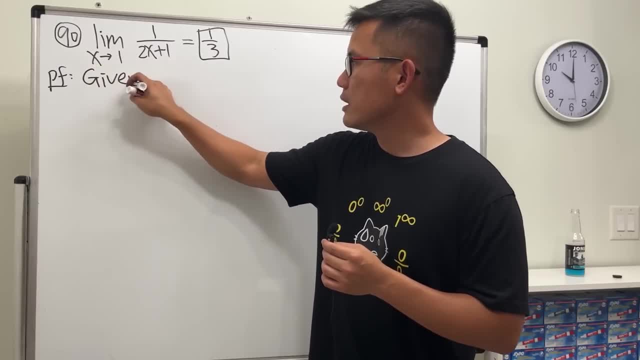 worry though I'll take up you guys PF. worry though I'll take up you guys PF. first given given Delta, so I give it up. first given given Delta, so I give it up. first given given Delta, so I give it up some quickness, you roll, then choose. 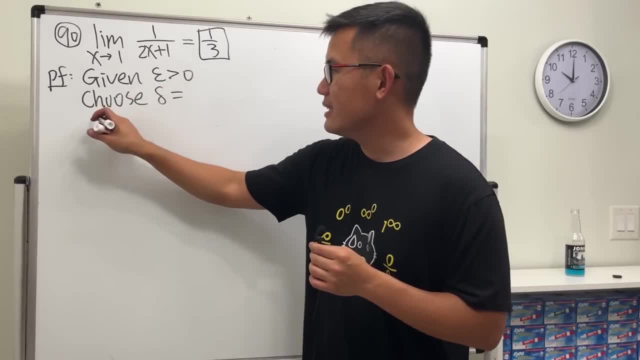 some quickness: you roll, then choose some quickness, you roll, then choose Delta, I don't know yet. then suppose Delta, I don't know yet. then suppose Delta, I don't know yet. then suppose absolute value of this minus that, so X. absolute value of this minus that, so X. 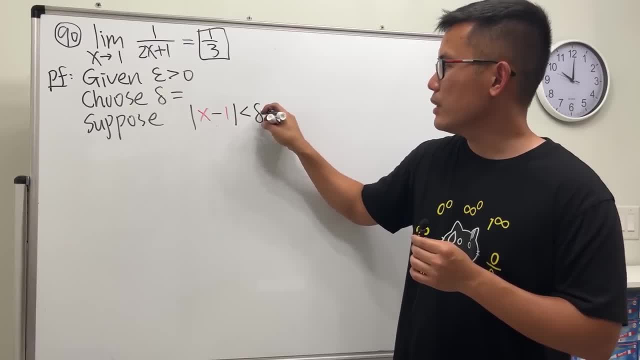 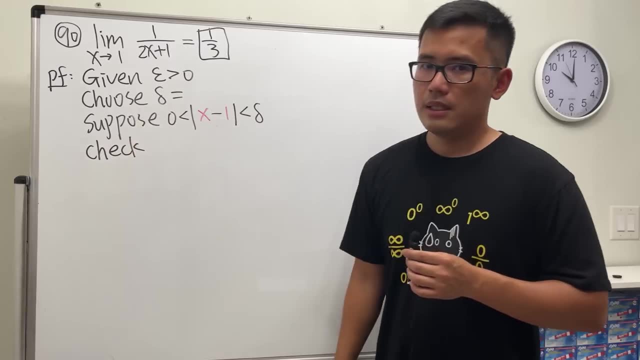 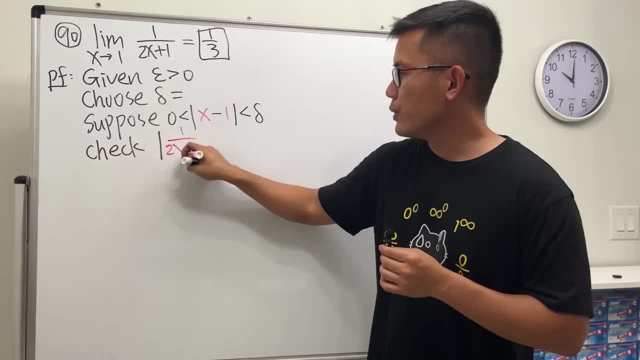 then we want to check: okay, absolute value function minus the limit, so we value function minus the limit, so we value function minus the limit. so we have 1 over 2x minus 1, so 2x plus 1. have 1 over 2x minus 1, so 2x plus 1. 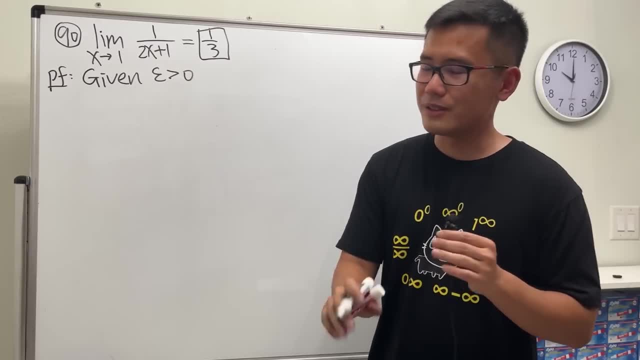 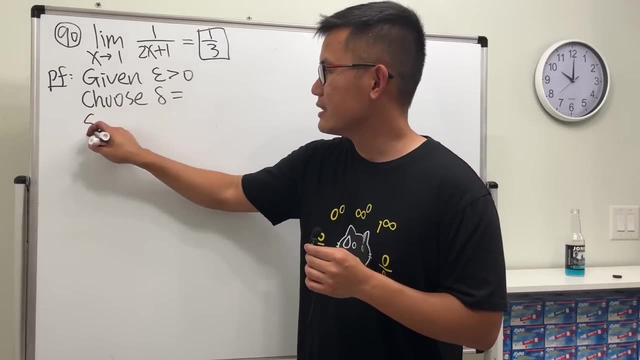 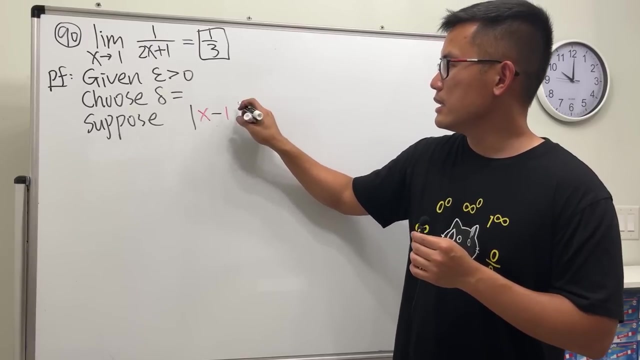 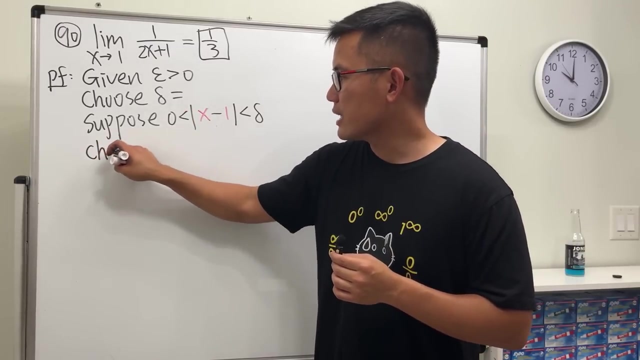 given delta, sorry, given epsilon greater than zero, then choose delta. i don't know yet. then suppose absolute value of this minus that. so x minus one is less than delta and greater than zero. then we want to check. okay, absolute value function minus the limit. so we have one. 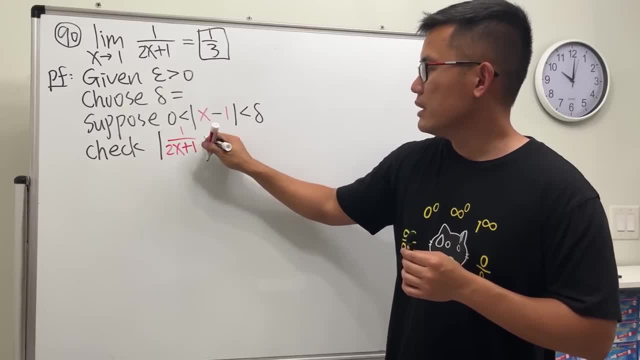 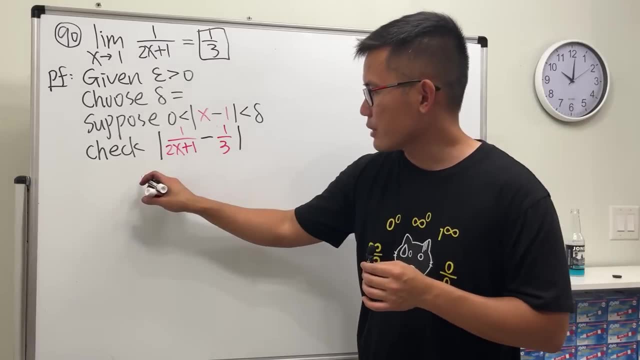 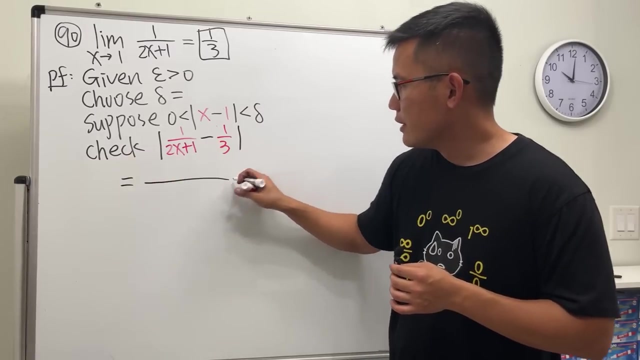 over two x minus, sorry, two x plus one minus one over three. right now let's just get the common denominator all the good stuff. so just put it down right here, maybe more space. okay, so three right here, minus right, and now just distribute: so minus two x, and then 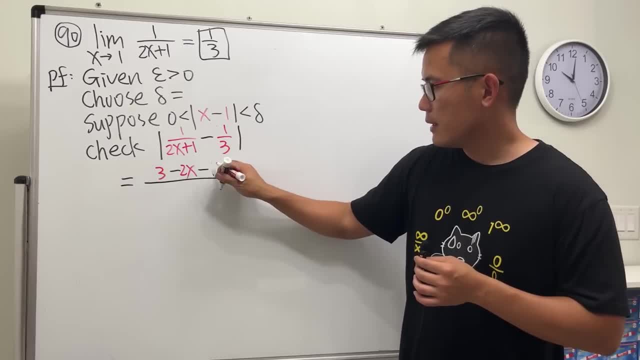 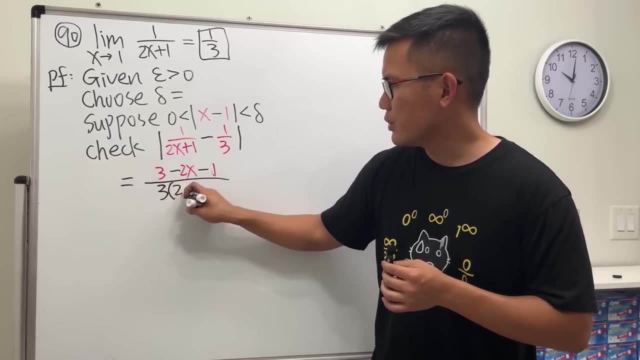 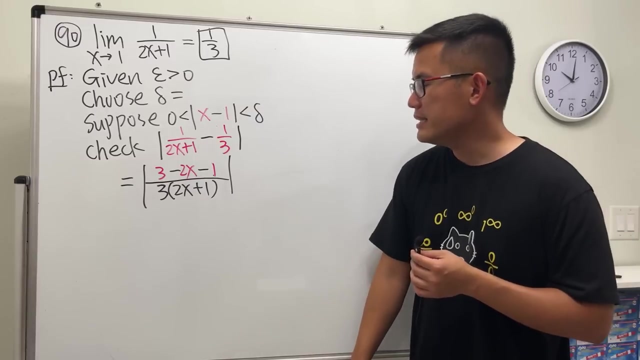 minus one. okay, and then on the bottom i'm just going to write this: three, three times two x plus one, yeah, something like this. hopefully you guys are okay with it: absolute value, all right, okay, three minus one is two, and then we can factor negative two. so this right here becomes: 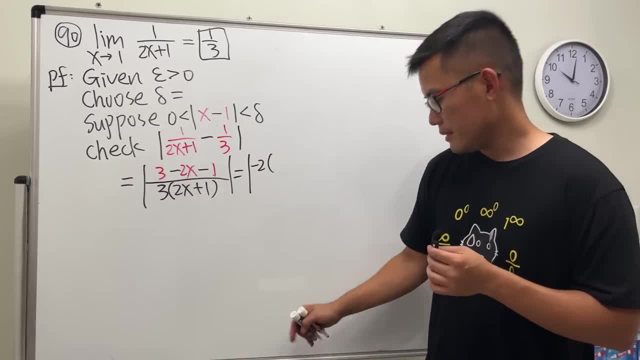 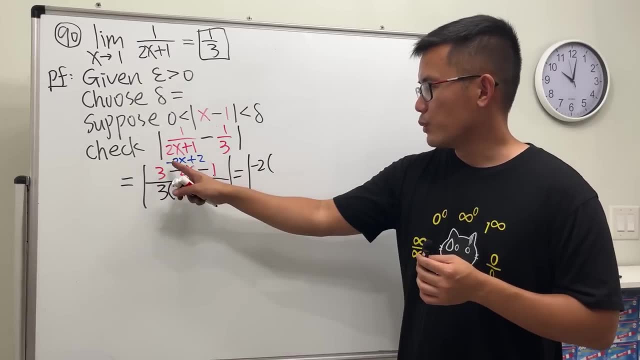 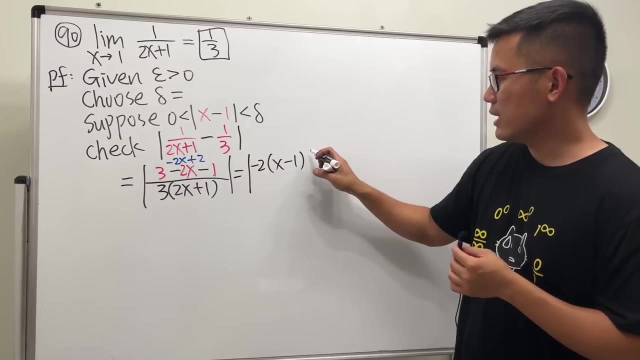 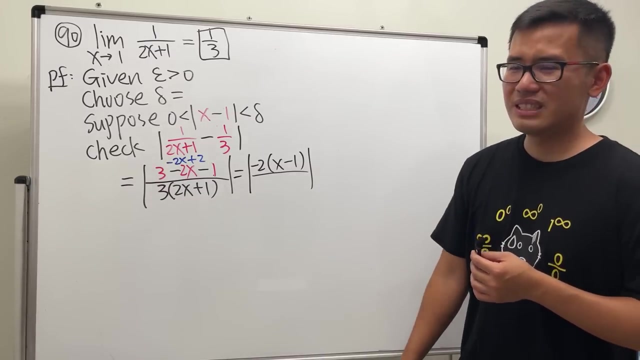 absolute value negative two, and then this is negative two. x plus two. yeah, so when we factor out a negative two, this becomes x minus minus one. yeah, so far, so good. we see that, huh, and then, um, the bottom is just that i can't really do too much. 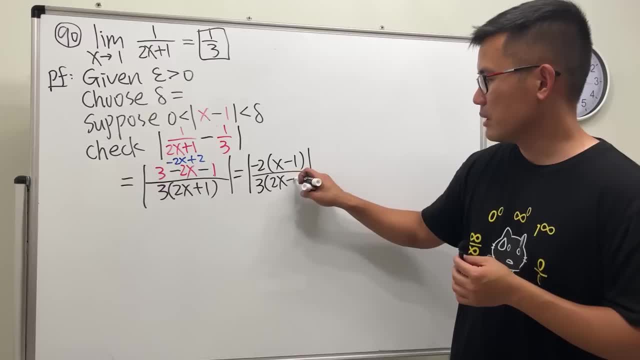 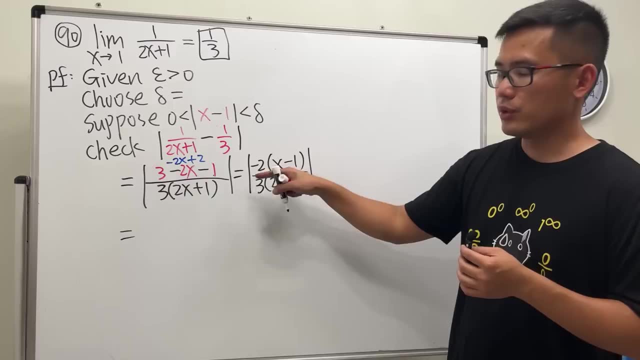 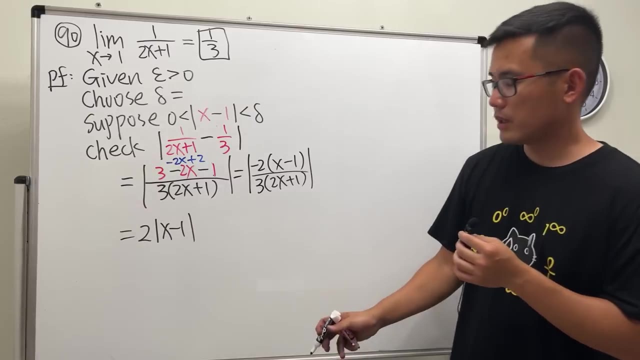 so i'm just going to keep it as that. so three, two x plus one. now break this apart: absolute value of the top and absolute value of the two. just negative two, just two, right, so we have two and absolute value, and then x minus one, okay, and then we have this on the bottom: 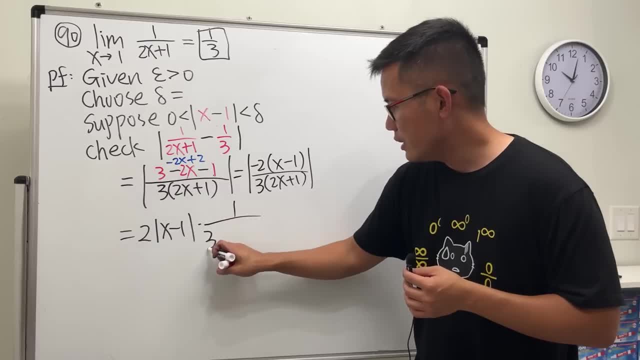 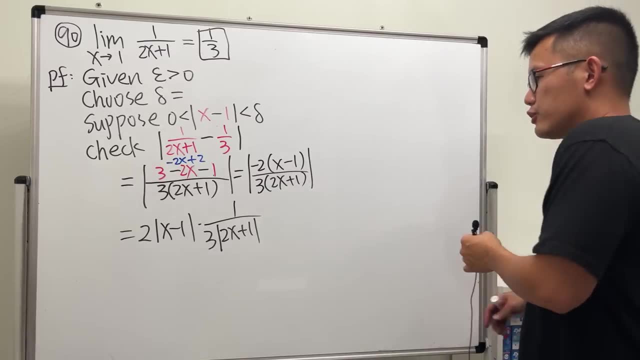 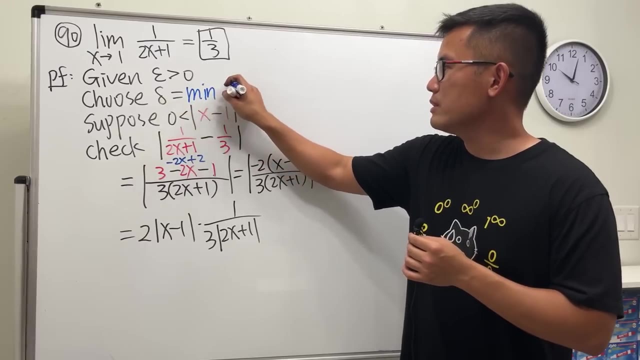 put a three on the outside, so one over three, and then absolute value of this: two x plus one. all right, so that's the algebra that we have so far. you know the deal come here: minimum 1.7. no, no, please don't, don't do that. 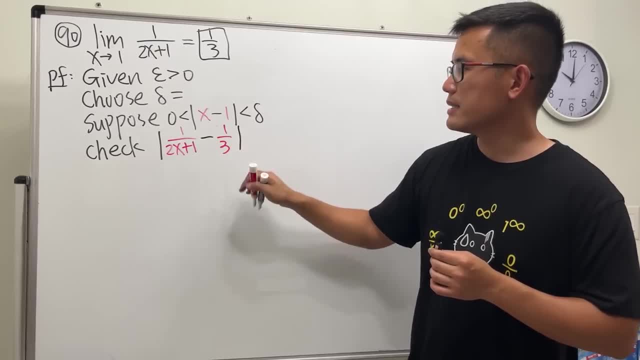 have 1 over 2x minus 1. so 2x plus 1 minus 1 over 3 right now. let's just get minus 1 over 3 right now. let's just get minus 1 over 3 right now. let's just get the common denominator, all the good. 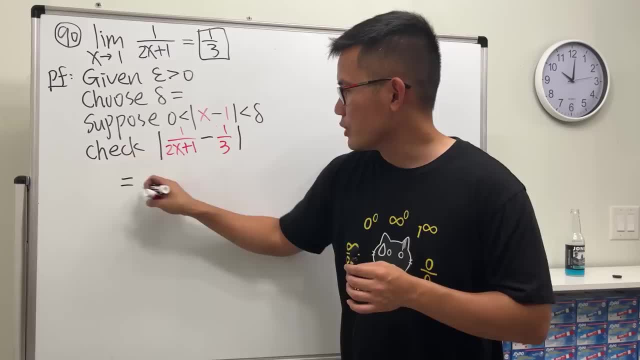 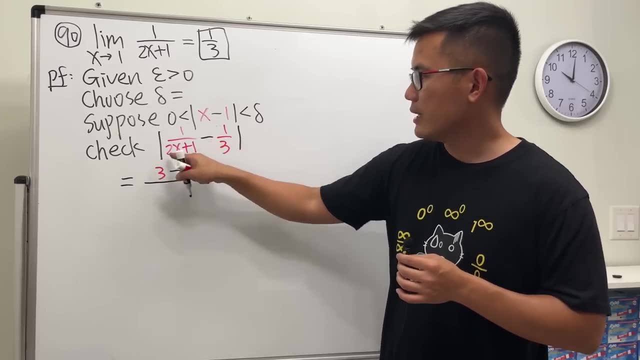 the common denominator, all the good, the common denominator, all the good stuff. so just put it down right here stuff. so just put it down right here stuff. so just put it down right here. maybe any more space, okay. maybe any more space, okay. maybe any more space, okay. so three right here, minus right, and now 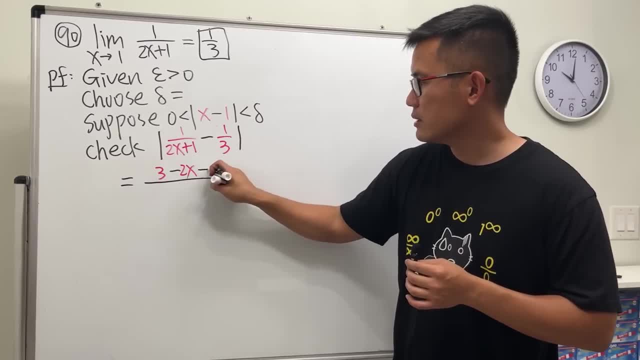 so three right here, minus right. and now so three right here, minus right. and now just distribute, so minus 2x. and then just distribute, so minus 2x, and then just distribute so minus 2x, and then minus 1, okay, and then on the bottom I'm. 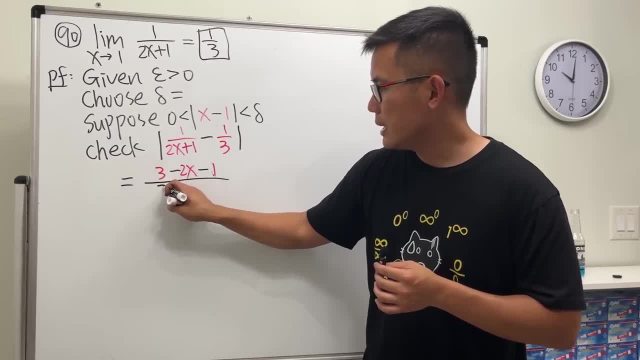 minus 1, okay, and then on the bottom, I'm minus 1, okay. and then on the bottom, I'm just going to write yes 3 times 2x plus. just going to write yes 3 times 2x, plus. just going to write yes 3 times 2x plus 1. yeah, someone like this, hopefully you. 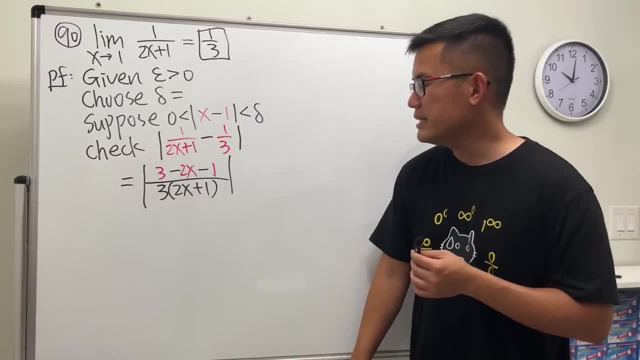 1. yeah, someone like this, hopefully you. 1. yeah, someone like this, hopefully you guys are okay with it. that's the value. guys are okay with it. that's the value. guys are okay with it. that's the value, alright, okay. 3 minus 1 is 2, and then we 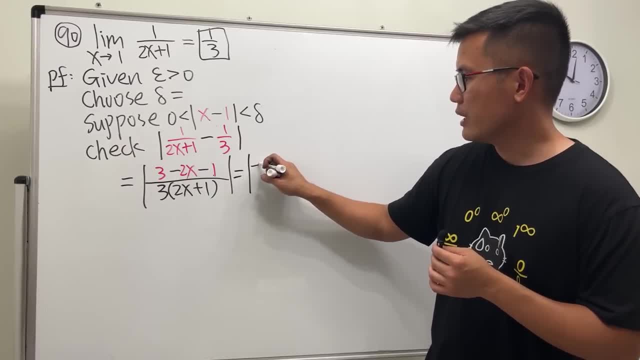 alright, okay, 3 minus 1 is 2. and then we: alright, okay, 3 minus 1 is 2, and then we can factor negative 2. so this right, it can factor negative 2. so this right, it can factor negative 2. so this right, it becomes absolutely negative 2. and then 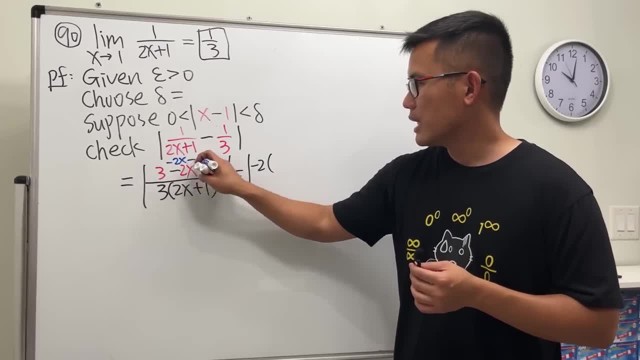 becomes absolutely negative 2, and then becomes absolutely negative 2, and then this is negative 2 X plus 2. yeah. so when this is negative 2 X plus 2, yeah. so when this is negative 2, X plus 2, yeah. so when we factor out a negative 2, this becomes. 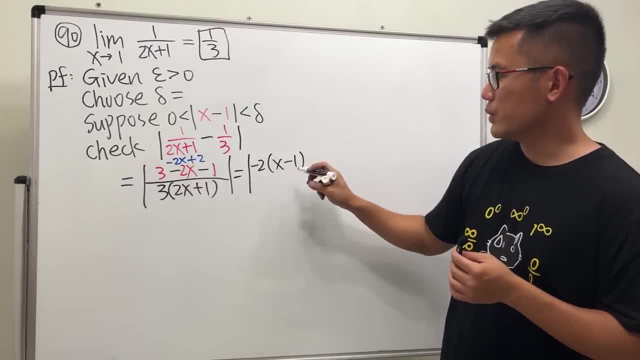 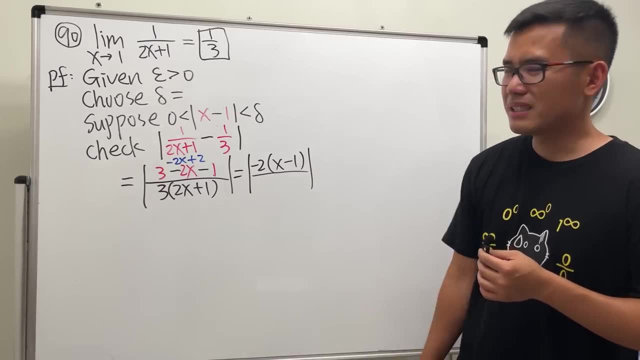 we factor out a negative 2, this becomes. we factor out a negative 2, this becomes X minus 1. yeah, so far, so good. we see X minus 1. yeah, so far, so good. we see X minus 1. yeah, so far, so good. we see that, huh, and then the bottom is just: I. 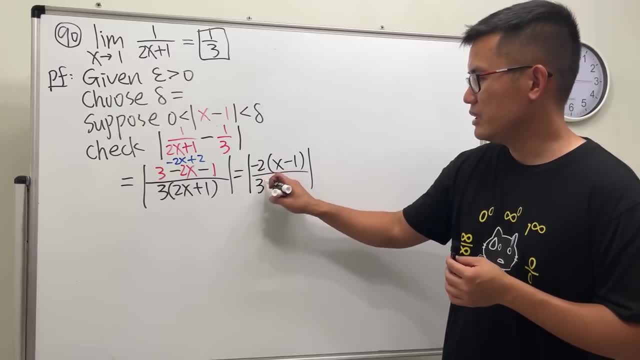 that huh. and then the bottom is just: I that huh. and then the bottom is just: I can't really do too much huh, so I'm can't really do too much huh, so I'm can't really do too much huh, so I'm just gonna keep it as that. so it's 3, 2 X. 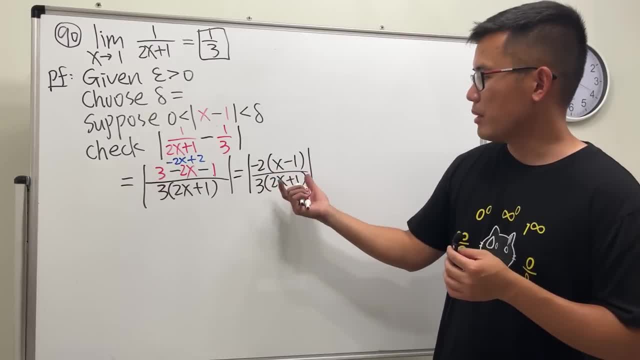 just gonna keep it as that. so it's 3, 2 X. just gonna keep it as that. so it's 3, 2 X plus 1. now break this apart after the plus 1. now break this apart after the plus 1. now break this apart after the photo of the top and absolute value of: 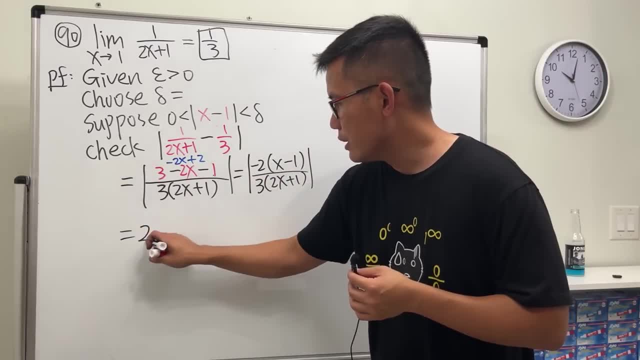 photo of the top and absolute value of photo of the top and absolute value of a: 2- just negative 2, just 2, right, so we a 2- just negative 2, just 2, right, so we a 2- just negative 2, just 2, right, so we have 2 and the absolute value. and then 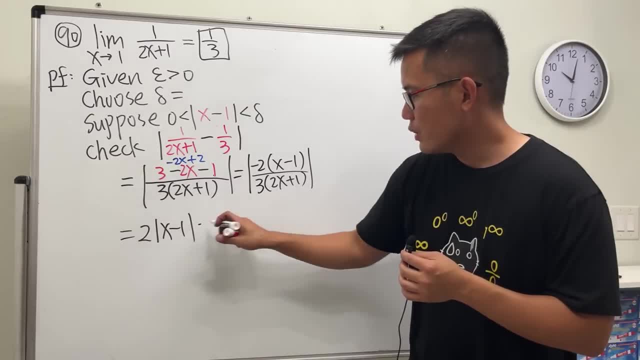 have 2 and the absolute value, and then have 2 and the absolute value and then X minus 1- okay. but then we have this on X minus 1, okay. but then we have this on X minus 1- okay. but then we have this on the bottom: put a string on outside, so 1. 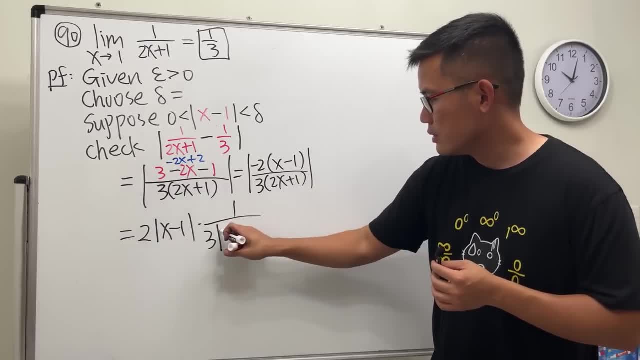 the bottom put a string on outside, so 1. the bottom put a string on outside, so 1 over 3. and the absolute value of this, 2 over 3, and the absolute value of this 2 over 3, and the absolute value of this 2 X plus 1. all right, so that's the algebra. 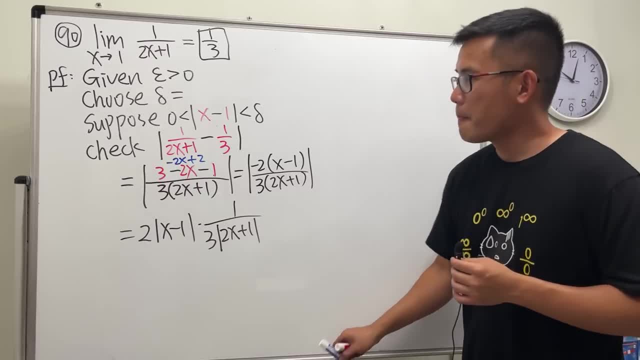 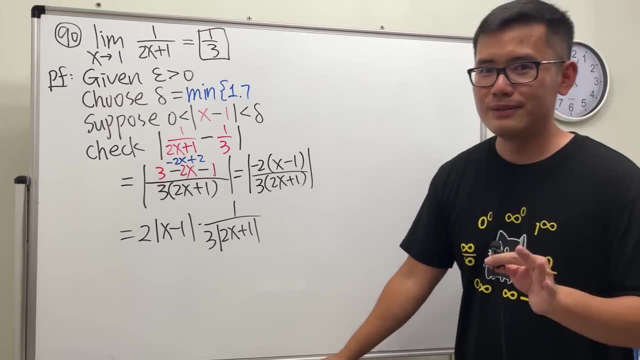 X plus 1, all right. so that's the algebra: X plus 1, all right. so that's the algebra that we have so far. you know the deal that we have so far. you know the deal that we have so far. you know the deal: come here: minimum 1.7. no, no, please don't. 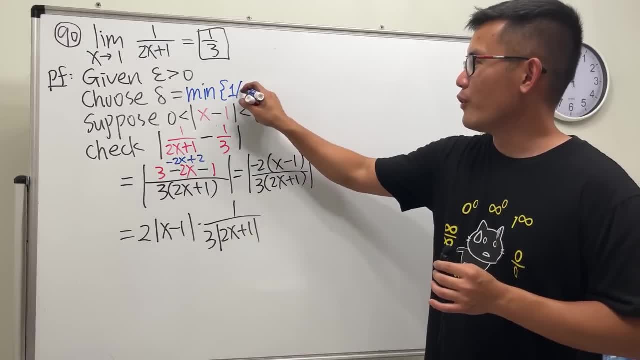 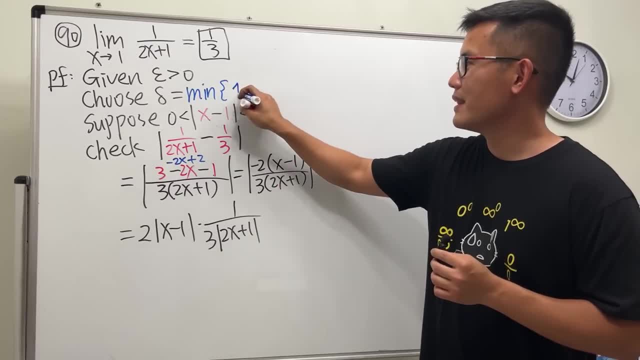 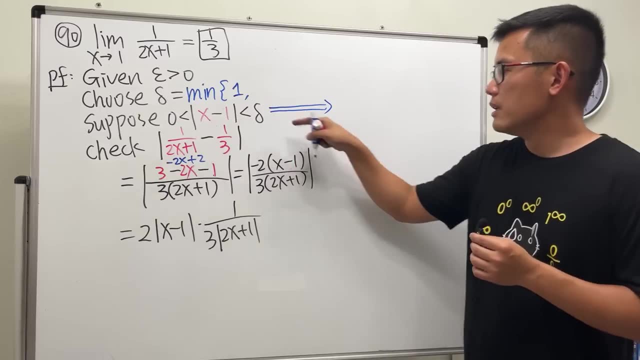 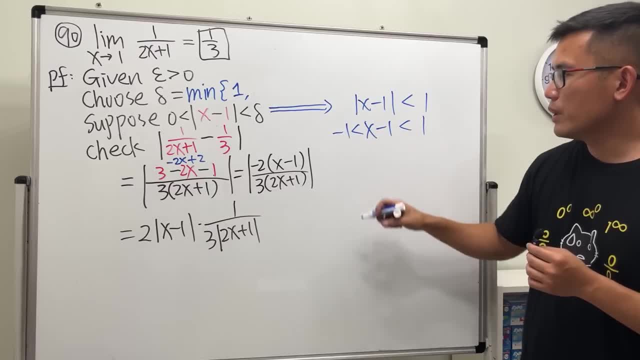 minus 1 is less than 1, open it. we get X minus 1 is less than 1, open it. we get X minus 1. it's in between of 1 here and minus 1. it's in between of 1 here and minus 1, it's in between of 1 here, and then put a negative 1 here and then just 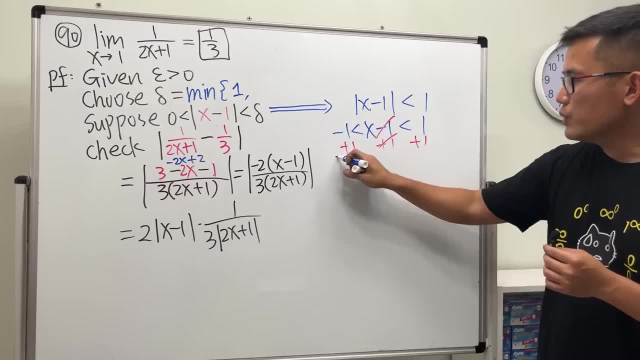 then put a negative 1 here, and then just then put a negative 1 here, and then just add 1 to everybody. so we see that's 0, add 1 to everybody. so we see that's 0, add 1 to everybody. so we see that's 0, and then that's X, and then I'm trying. 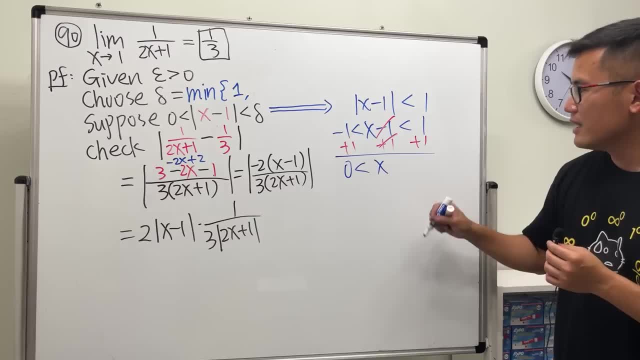 and then that's X, and then I'm trying, and then that's X, and then I'm trying to get to the huh. but let's, let's do the to get to the huh, but let's, let's do the to get to the huh, but let's, let's do the things that we do earlier. 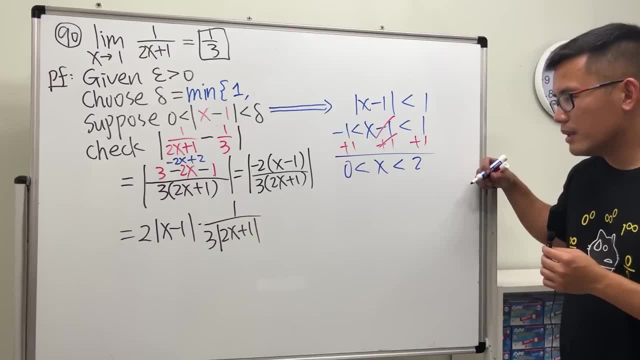 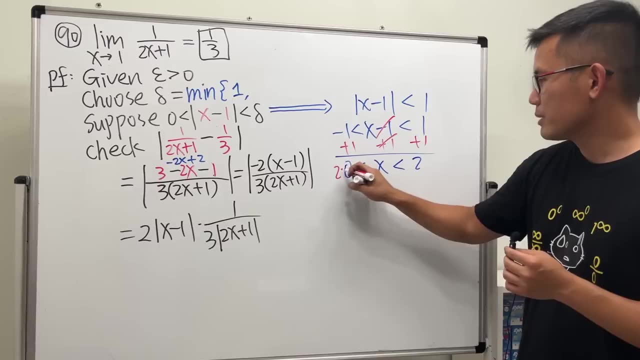 things that we do earlier, things that we do earlier: 2- okay, okay, fine, I need a 2x, so let's 2- okay, okay, fine, I need a 2x, so let's 2, okay, okay, fine, I need a 2x. so let's multiply everybody by 2, so multiply by 2. 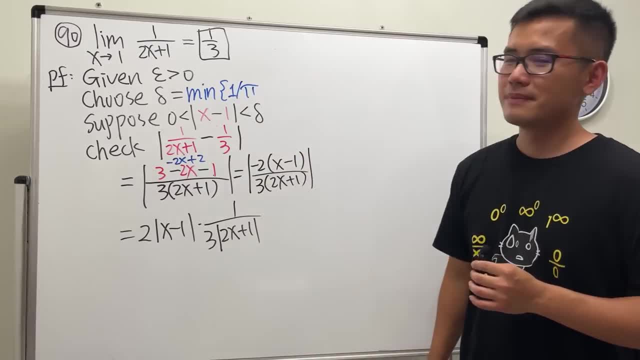 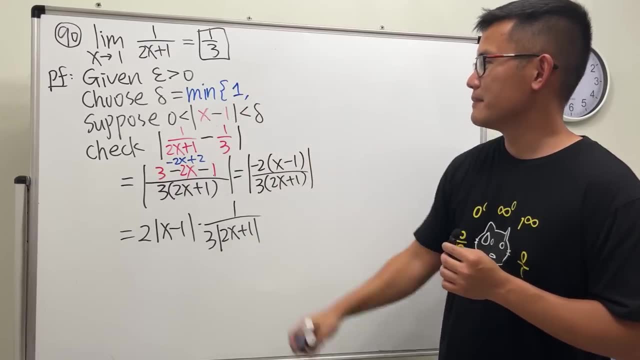 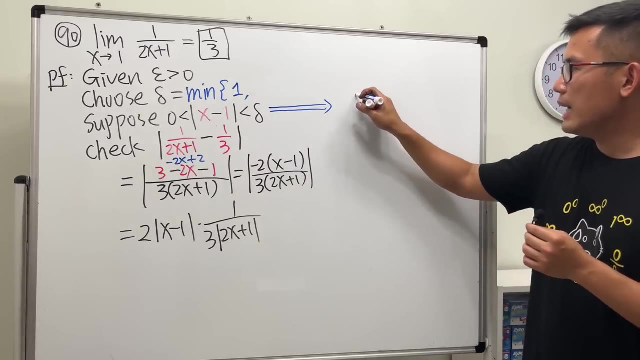 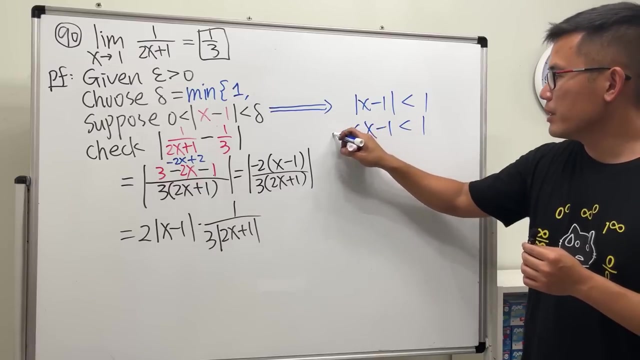 of course you should do one over pi, okay, okay, okay, okay, one. all right here. let's see, look at absolute value. of x minus one is less than one. open it, we get x minus one. it's in between of one here and then put a negative one here and then. 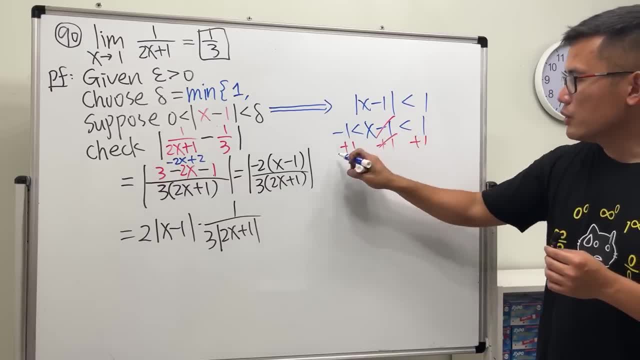 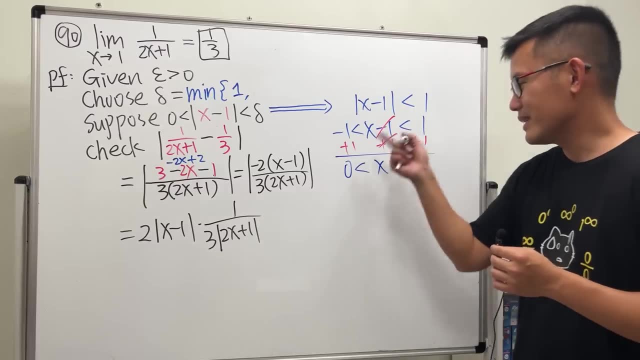 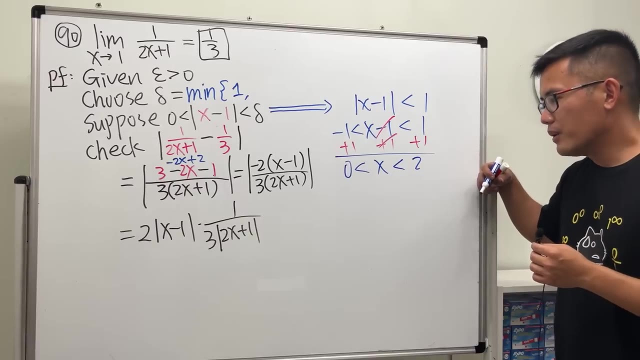 just add one to everybody so we see that's zero and then that's x, and then, oh, i'm trying to get to there, huh, but let's, let's do the things that we did earlier. uh, two, okay, okay, fine, i need a two x. so let's multiply everybody by two. so 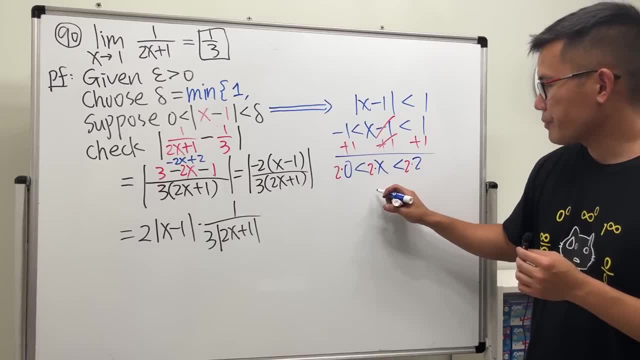 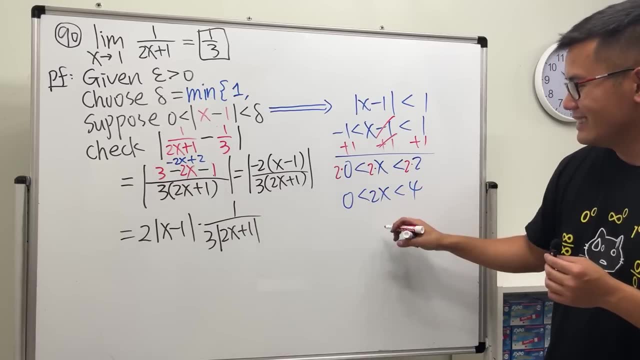 multiply by two, multiply by two, multiply by two, so two x is in between of zero, and then four, and then let's add one to everybody. uh, so yeah, one, one and one, things like this. pretty cool, i would say. so we have two x plus one. it's in between. 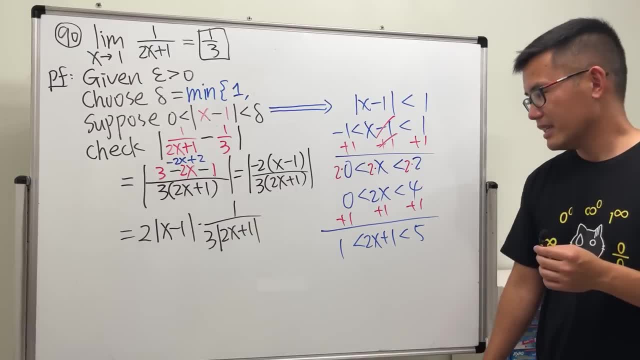 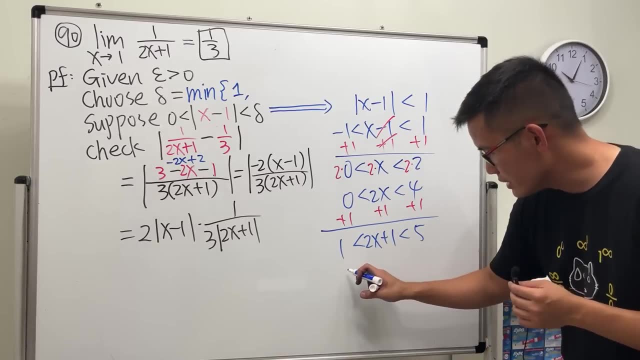 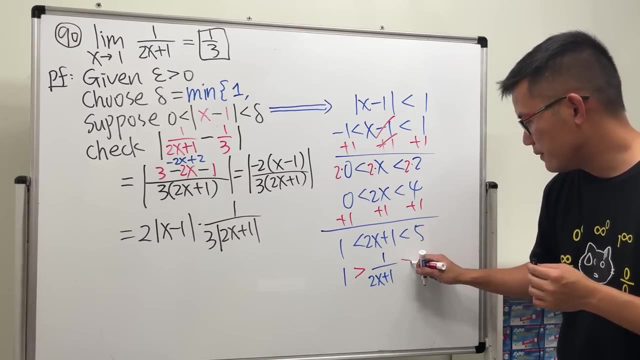 of one and five. what did we do earlier? we take the reciprocal first right. so we take the reciprocal- this is going to be one over one which is one, and flip one over two x plus one, and then flip and then also reciprocal, that which one has a bigger. 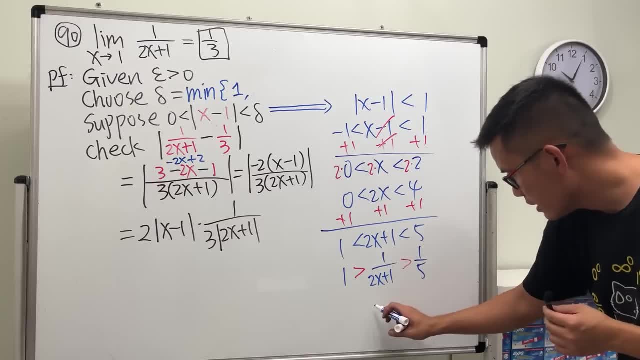 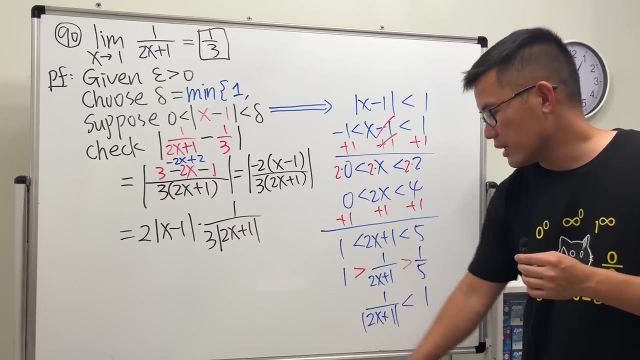 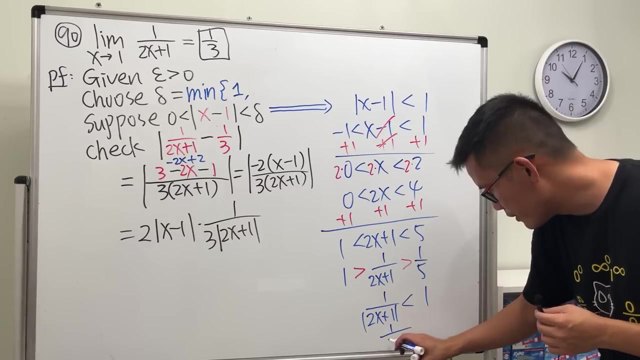 absolute value. this does so. this means one over two x plus one in the absolute value is less than one. really interesting, because we saw the one earlier too. yeah, and we want the street right there, huh. so let's just say that to have enough space. one over three absolute. 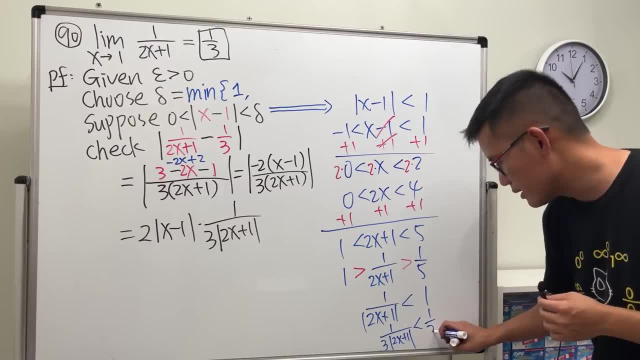 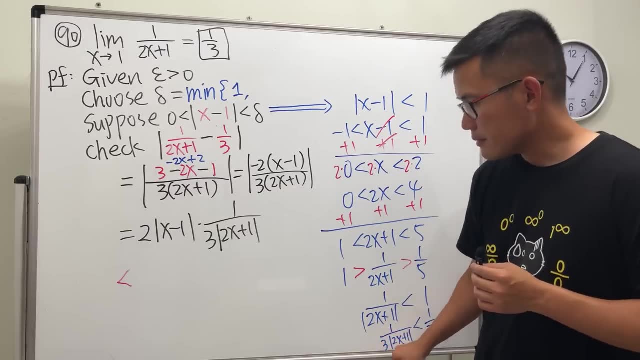 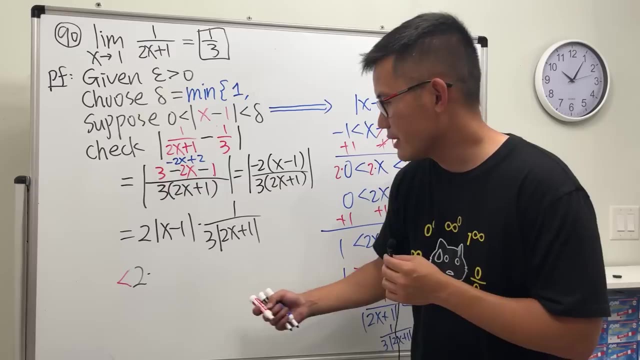 value: two x plus one is less than one third. okay, all right, this thing we have. the less than two is still two. this is less than delta. i forgot to say that earlier. i was too excited to work out that. all right, and this thing? let me just 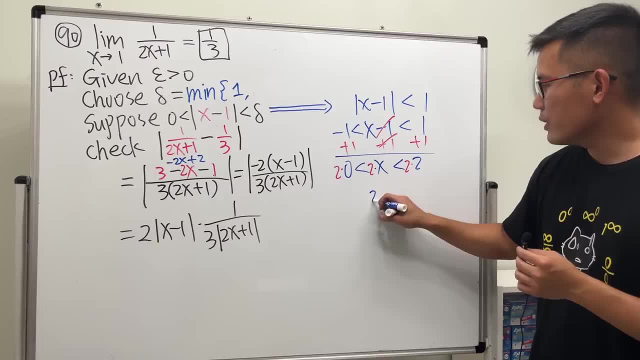 multiply everybody by 2, so multiply by 2. multiply everybody by 2, so multiply by 2. multiply by 2. multiply by 2, so 2x is in. multiply by 2, so 2x is in. multiply by 2, so 2x is in between of 0 and then 4, and then let's add 1 to. 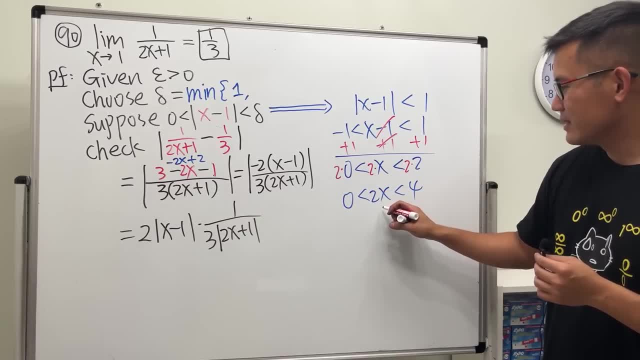 between of 0 and then 4, and then let's add 1 to between of 0 and then 4, and then let's add 1 to everybody. so yeah, 1, 1 and 1 everybody. so yeah, 1, 1 and 1. 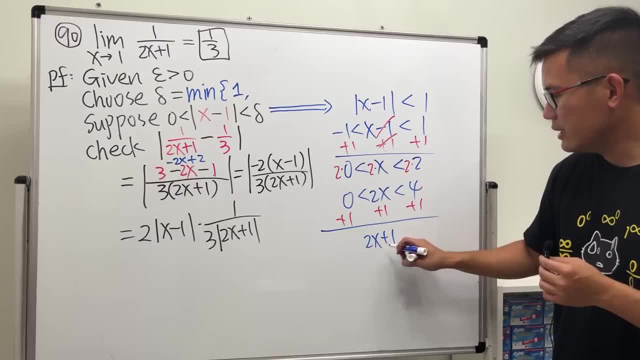 everybody. so yeah, 1, 1 and 1. things like this pretty cool, I'll say so. things like this pretty cool, I'll say so. things like this pretty cool, I'll say so. we have 2x plus 1. it's in between of 1. 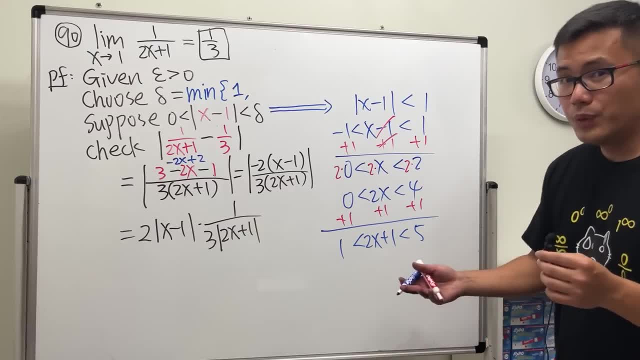 we have 2x plus 1. it's in between of 1. we have 2x plus 1. it's in between of 1 and 5. what did we do earlier? we take and 5. what did we do earlier? we take and 5. what did we do earlier we take that reciprocal first right. so we take. 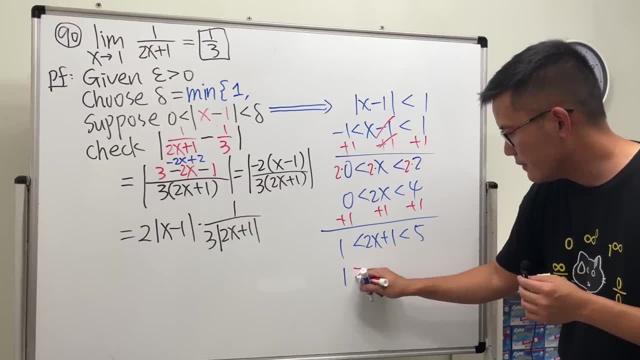 that reciprocal first right. so we take that reciprocal first right. so we take the reciprocal. this is gonna be 1 over the reciprocal. this is gonna be 1 over the reciprocal. this is gonna be 1 over 1, which is 1, and flip 1 over 2, X plus 1. 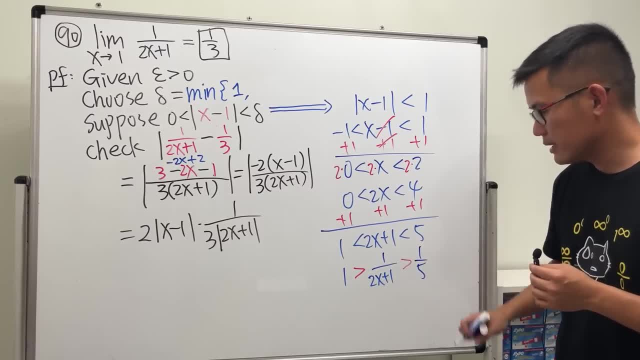 1, which is 1, and flip 1 over 2 X plus 1, 1, which is 1, and flip 1 over 2 X plus 1, and then flip, and then also reciprocal, and then flip, and then also reciprocal, and then flip, and then also reciprocal. that which one has a big gap for you. 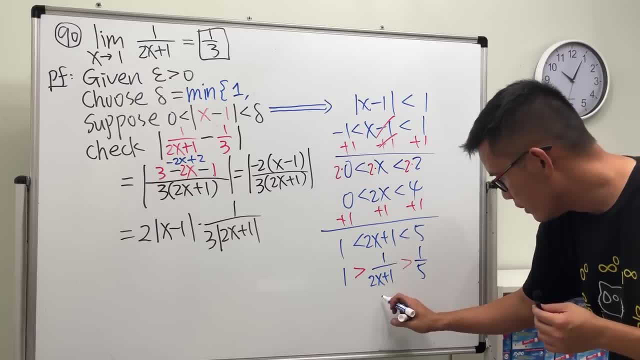 that which one has a big gap for you. that which one has a big gap for you. this does so. this means 1 over 2 X plus. this does so. this means 1 over 2 X plus this does so. this means 1 over 2 X plus 1. in the absolute value is less than 1. 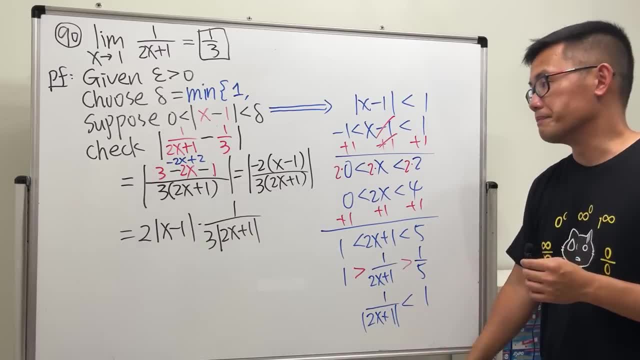 1 in the absolute value is less than 1. 1 in the absolute value is less than 1. really interesting up because we saw the really interesting up, because we saw the really interesting up, because we saw the one earlier too. yeah, and we want the. 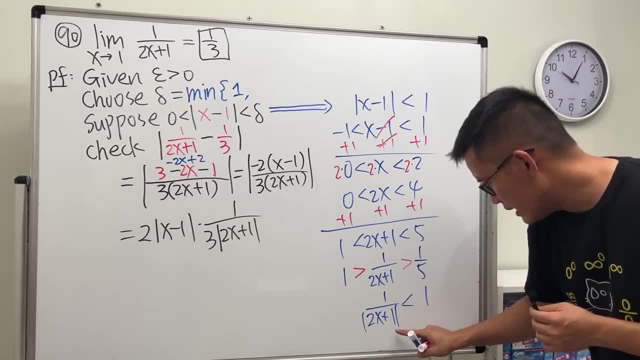 one earlier too. yeah, and we want the one earlier too. yeah, and we want the street right there, huh. so let's just say: street right there, huh. so let's just say street right there, huh. so let's just say that to have enough space. 1 over 3. 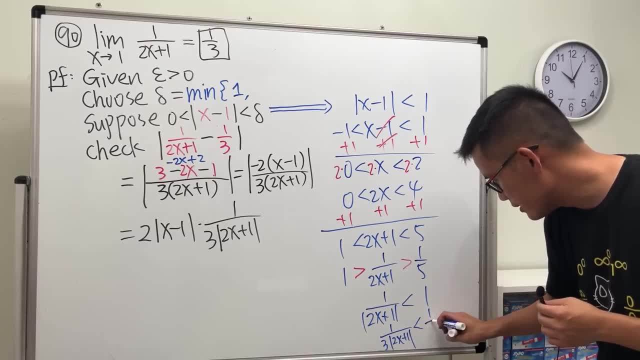 that to have enough space: 1 over 3. that to have enough space 1 over 3. absolute value: 2x plus 1 is less than 1. absolute value: 2x plus 1 is less than 1. absolute value: 2x plus 1 is less than 1. third, okay, all right, this thing we have. 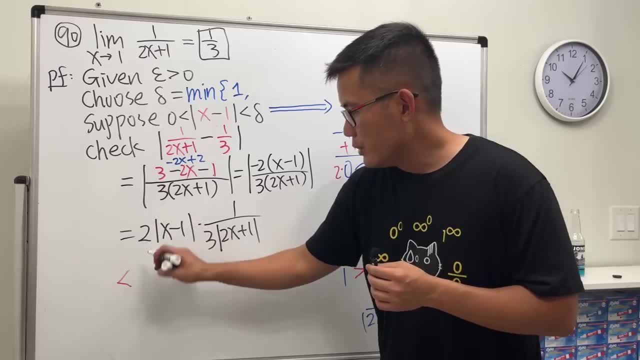 third: okay, all right, this thing we have. third: okay, all right, this thing we have. the lesson 2 is still 2. this is less than the lesson 2 is still 2. this is less than the lesson 2 is still 2. this is less than delta. I forgot to say that earlier. I. 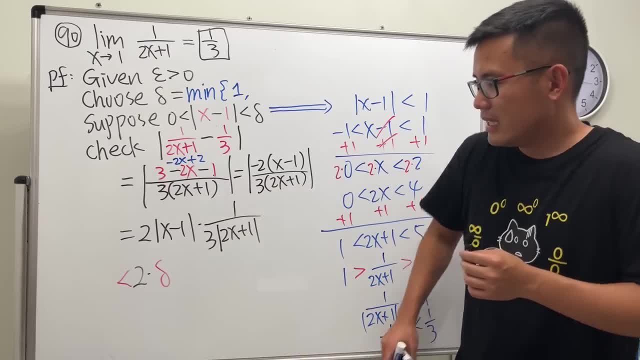 delta. I forgot to say that earlier I delta. I forgot to say that earlier I was too excited to work out that all right, was too excited to work out that all right, was too excited to work out that, all right. and this thing? let me just do like. 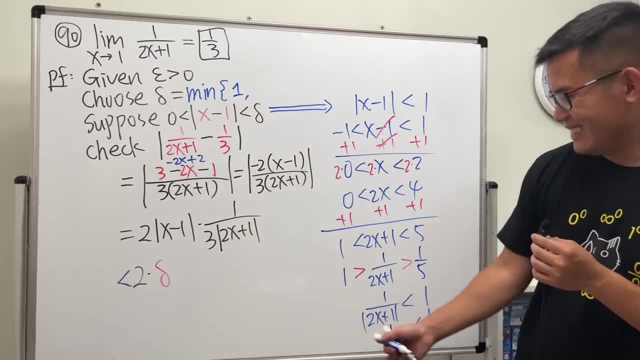 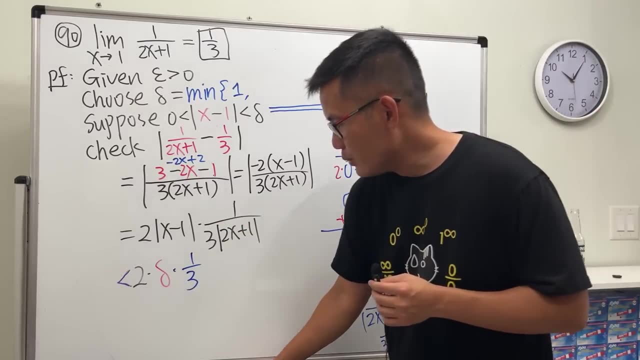 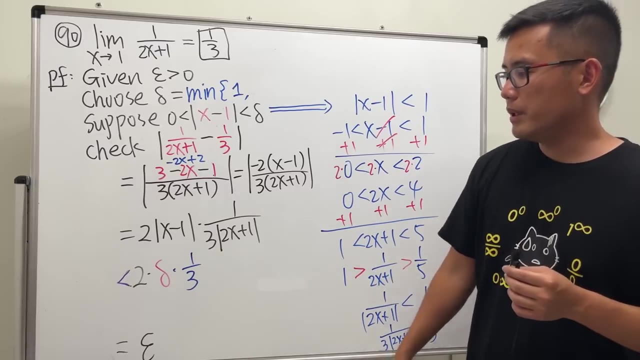 do like purple there. it's less than one over three, so multiply this and we get one over three. now, ladies and gentlemen, all the way, at the end we want to end up with epsilon. so what should we pick for? delta? we better have a delta. we better have an epsilon here, right? 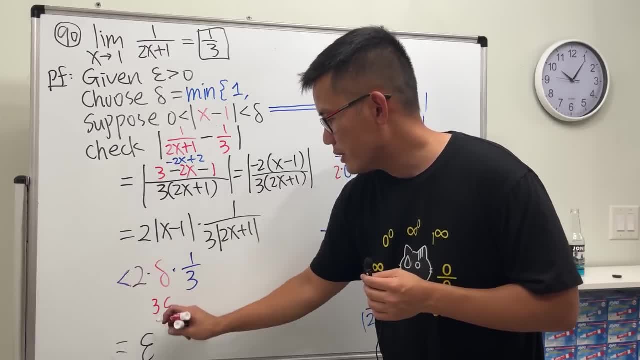 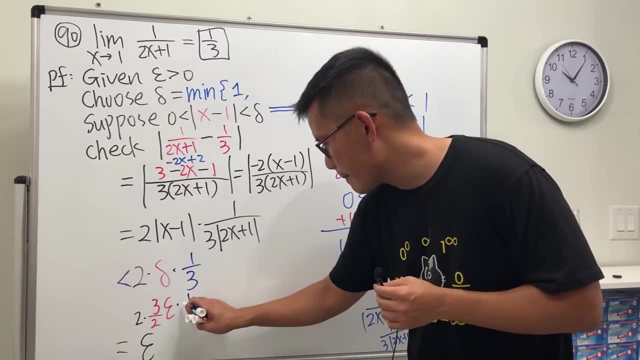 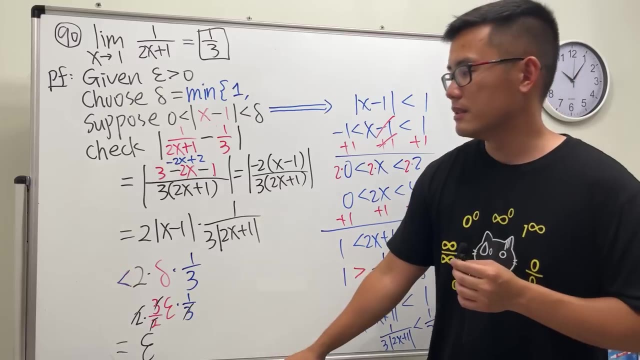 we divide it by three, so we better multiply by three. we multiply by two here, so we shall divide it by two, and when we have that, we can see: two and two cancel, three and three cancel, and we'll just end up with epsilon. and uh, delta is equal to that. 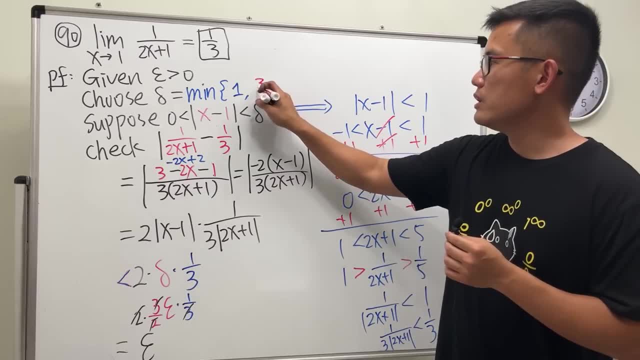 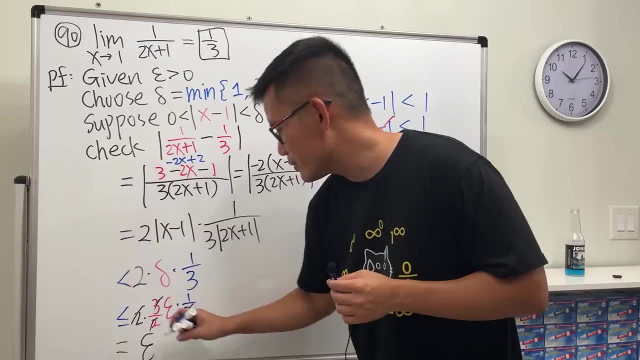 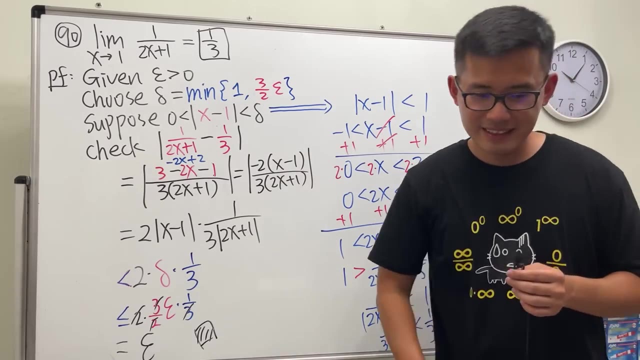 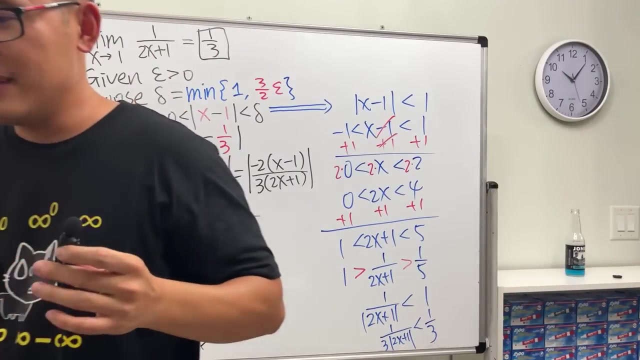 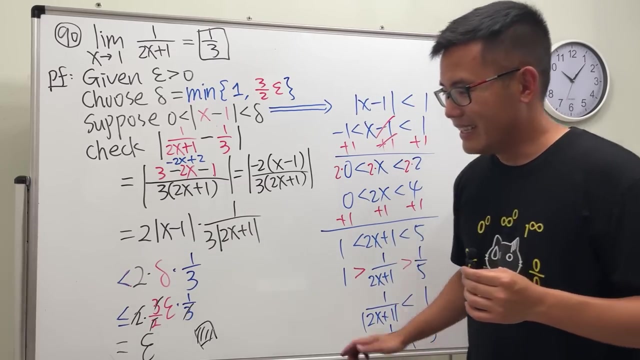 so we will come here and put down three over two epsilon and then hurry up, let's close this and then put down and then, yes, you think we are done. no, we have ten more pretty hard questions. okay, remount sum: are they any easier? uh, depends, they definitely look. 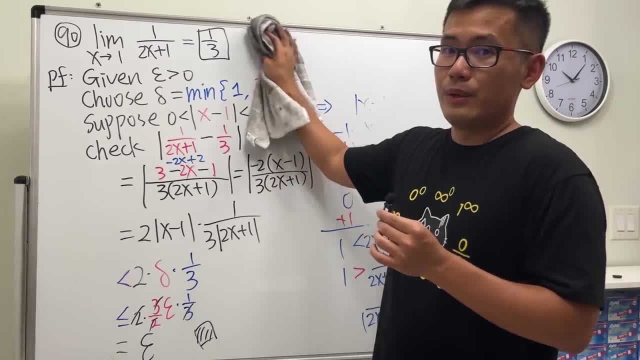 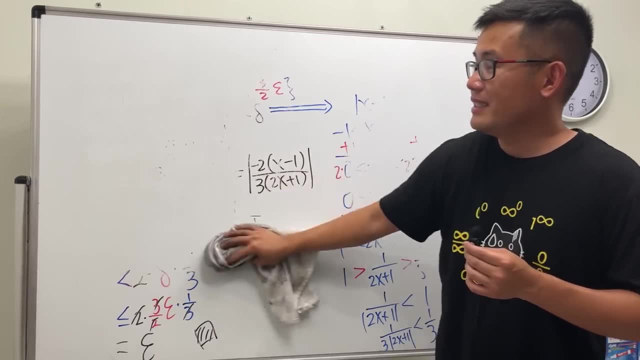 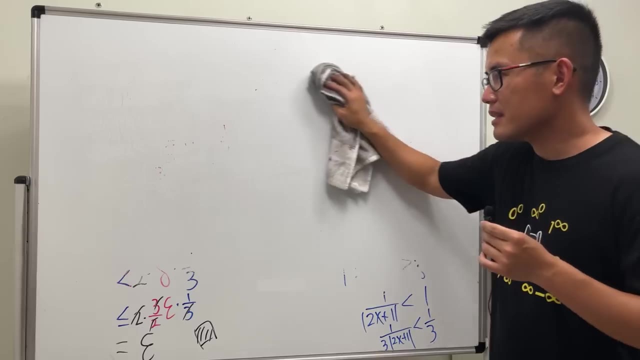 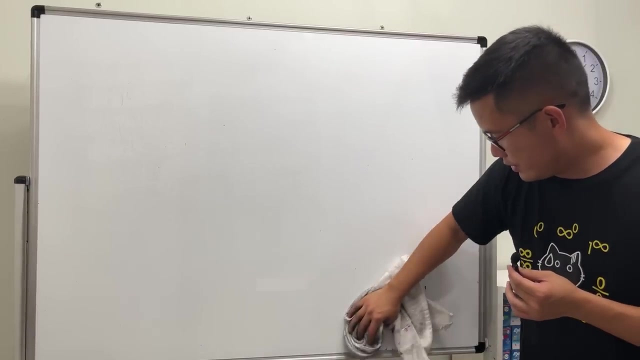 scarier because they are longer. you see this right here. they look like the question looks like this, but like the work is a lot for the remount sum for the definition of integral, pretty much um, the. the question is like that long and then the work is actually not bad. 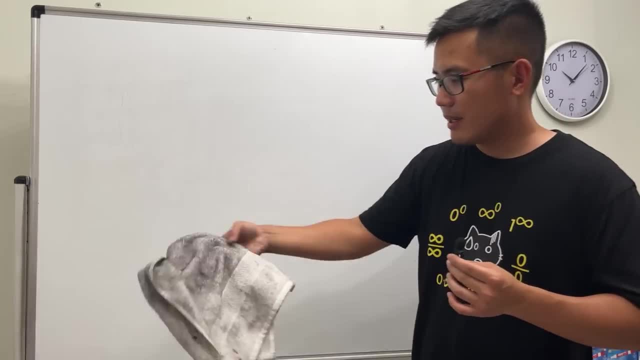 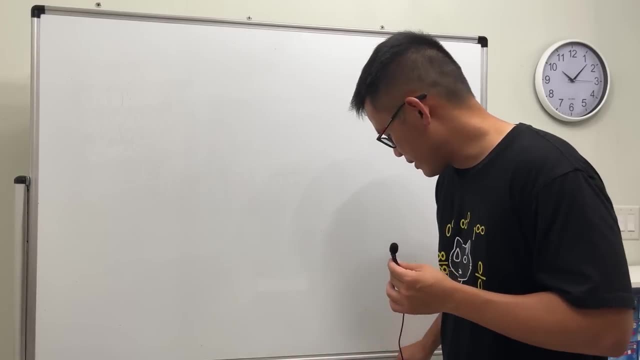 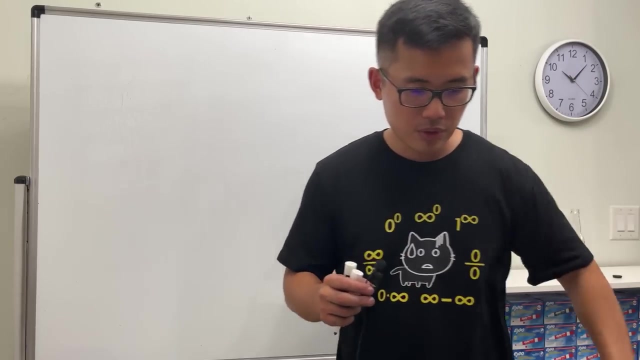 i'm going to simplify for you guys. right, i'm not going to over complicate the remount sum, because once you know what to look for, then, yeah, you know the deal already and i do have a very detailed explanation for remount sum as well. so 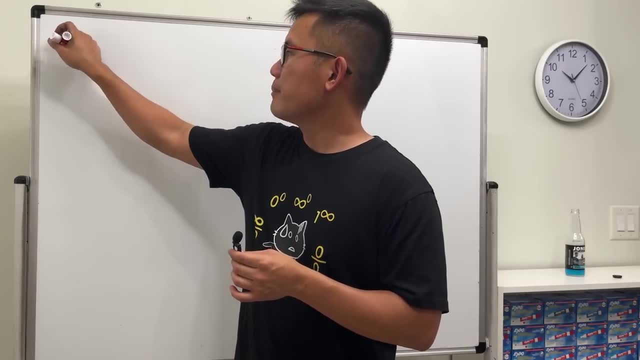 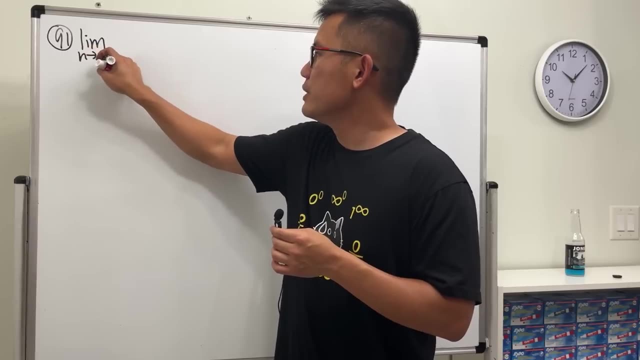 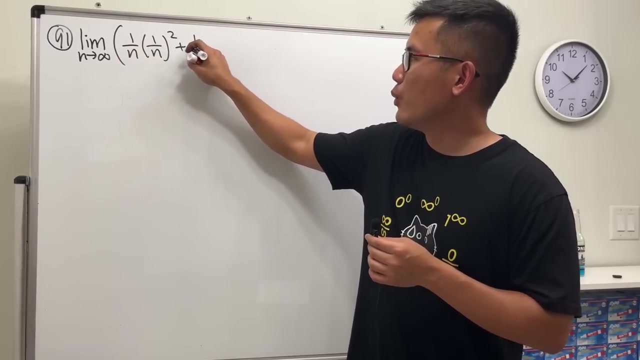 yeah, ladies and gentlemen, number 91 will come to a very, very long limit limit, as n goes to infinity ready. first one: 1 over n times 1 over n square. next one: 1 over n times 2 over n square. next one: 1 over n. 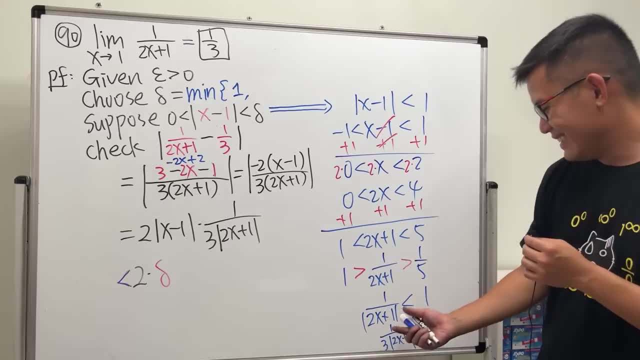 and this thing let me just do like. and this thing let me just do like: purple. yeah, it's less than 1 over 3 purple. yeah, it's less than 1 over 3 purple. yeah, it's less than 1 over 3. so multiply this and we can 1 over 3 now. 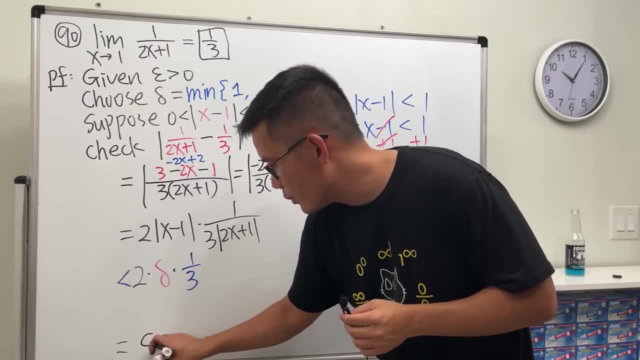 so multiply this, and we can 1 over 3 now. so multiply this and we can 1 over 3 now. ladies and gentlemen, all the way at the ladies and gentlemen, all the way at the ladies and gentlemen, all the way at the end. we want to end up with epsilon. so 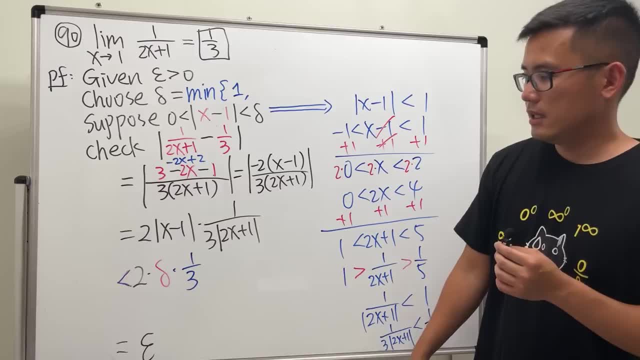 end, we want to end up with epsilon. so end, we want to end up with epsilon. so what should we pick for Delta? we better. what should we pick for Delta? we better. what should we pick for Delta? we better, have a Delta. we put up the epsilon here. 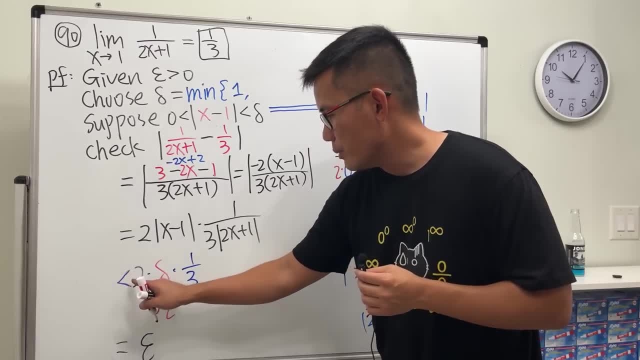 have a Delta. we put up the epsilon. here. have a Delta, we put up the epsilon here, right, we divided by 3, so we better, right, we divided by 3, so we better, right, we divided by 3, so we better multiply by 3. we multiply by 2 here, so we. 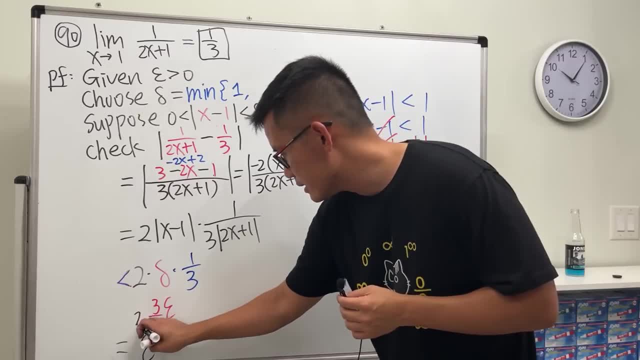 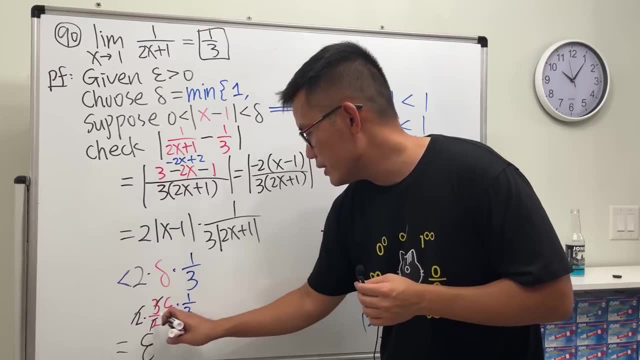 multiply by 3, we multiply by 2 here, so we multiply by 3, we multiply by 2 here, so we shall divided by 2, and when we have shall divided by 2, and when we have shall divided by 2, and when we have that, we can see 2 and 2, can. so 3 and 3. 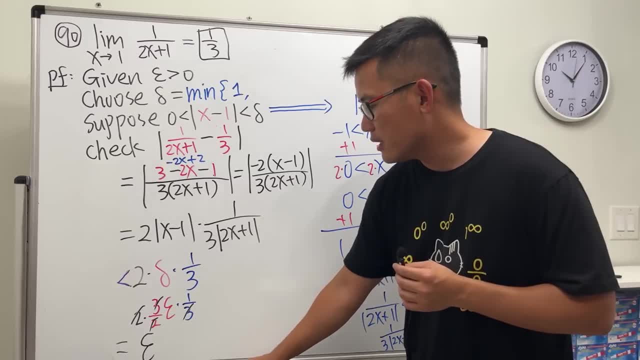 that we can see 2 and 2, can, so 3 and 3. that we can see 2 and 2, can, so 3 and 3: cancel, and we'll just end up with cancel and we'll just end up with cancel and we'll just end up with epsilon and Delta is equal to that, so we 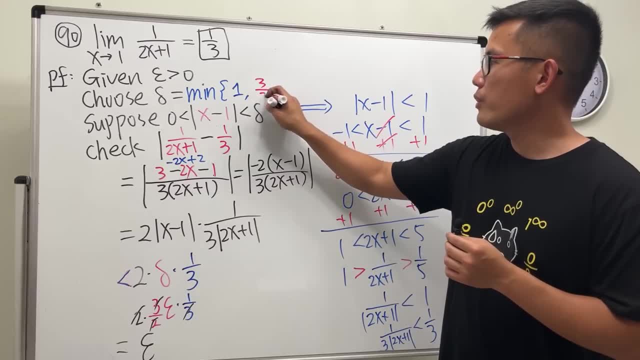 epsilon and Delta is equal to that. so we epsilon and Delta is equal to that. so we will come here and put down 3 over 2. will come here and put down 3 over 2. will come here and put down 3 over 2 epsilon and then hurry up. let's close. 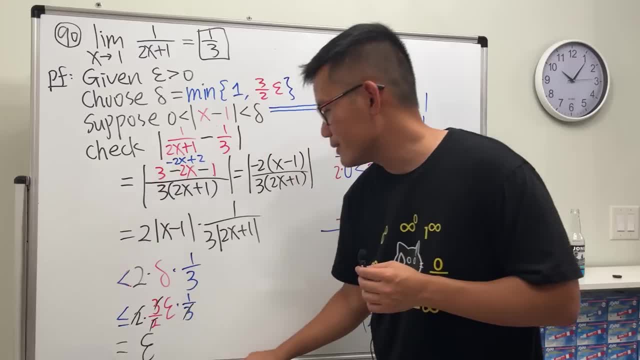 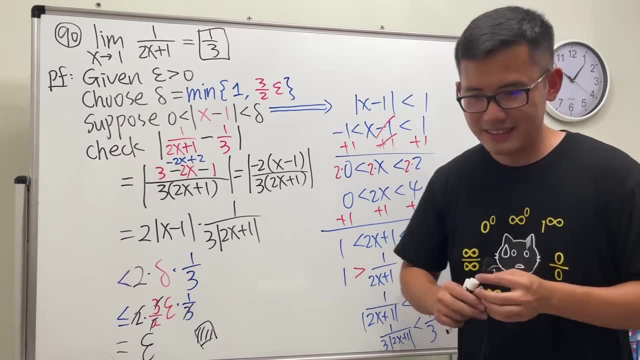 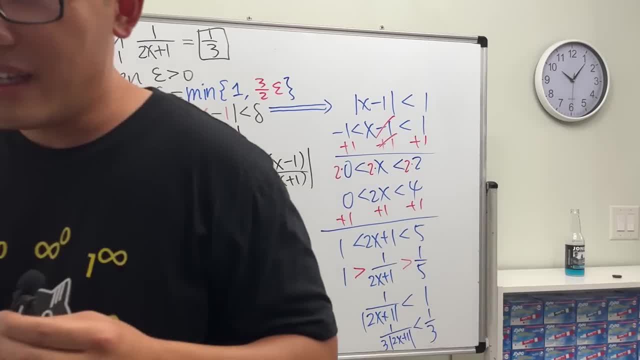 whoo you think we're done? no, we have 10. whoo you think we're done? no, we have 10 more pretty hard questions. why are they more pretty hard questions? why are they more pretty hard questions? why are they remain some? are they any easier? depends. 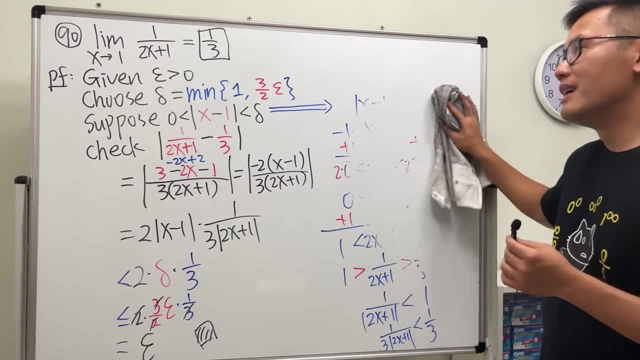 remain- some are they any easier? depends- remain. some are they any easier? depends. they definitely look scarier because they definitely look scarier, because they definitely look scarier, because they are longer. you see this right here. they are longer. you see this right here. they are longer. you see this right here. they look like. the question looks like. 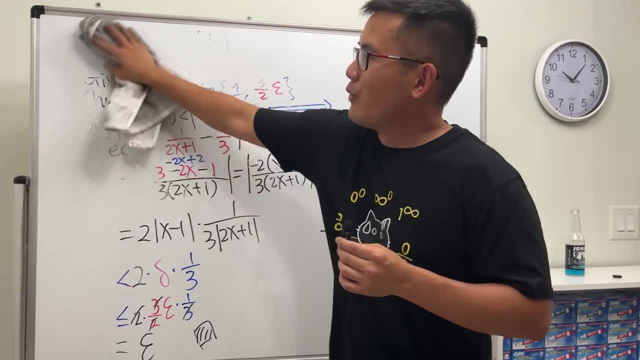 they look like the question looks like. they look like the question looks like this. but I go work. it's a lot this, but I go work. it's a lot this, but I go work. it's a lot for the remote son for the in definition. for the remote son for the in definition. 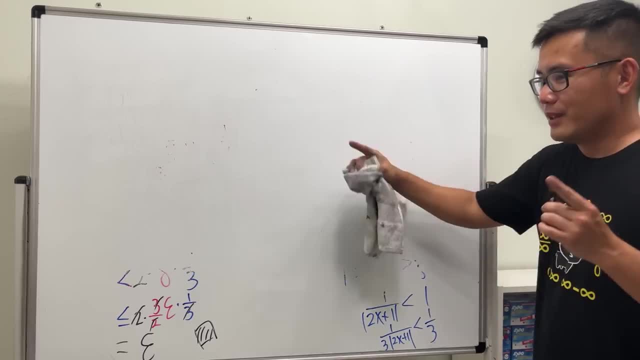 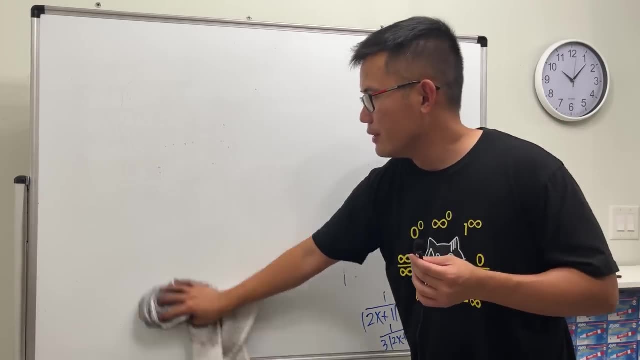 for the remote son, for the in definition of integral. pretty much the questions of integral. pretty much the questions of integral. pretty much the questions like that long and then the work is like that long and then the work is like that long and then the work is actually not bad. I'm going to simplify. 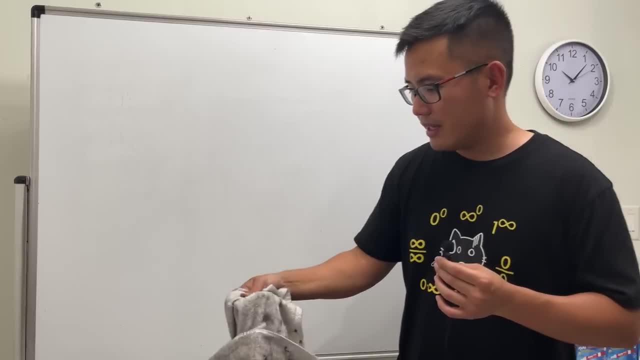 actually not bad. I'm going to simplify- actually not bad. I'm going to simplify for you guys, right? I mean I'm going to for you guys, right? I mean I'm going to for you guys, right? I mean I'm going to overcomplicate a remote song because 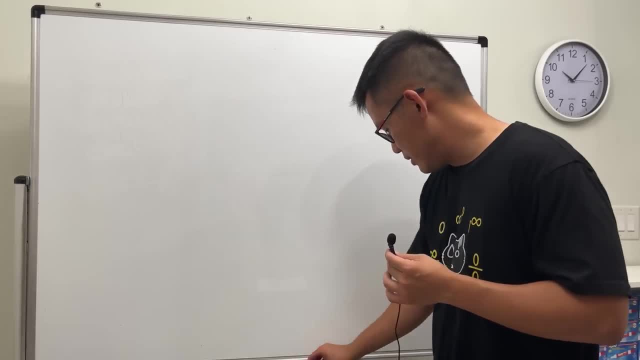 overcomplicate a remote song because overcomplicate a remote song? because once you know what to look for, then yeah. once you know what to look for, then yeah. once you know what to look for, then yeah, you know that you already. you know that you already. 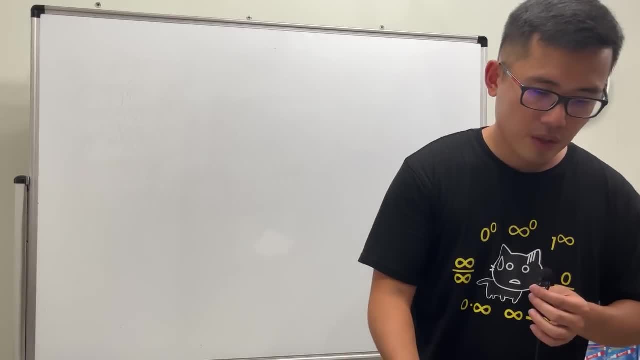 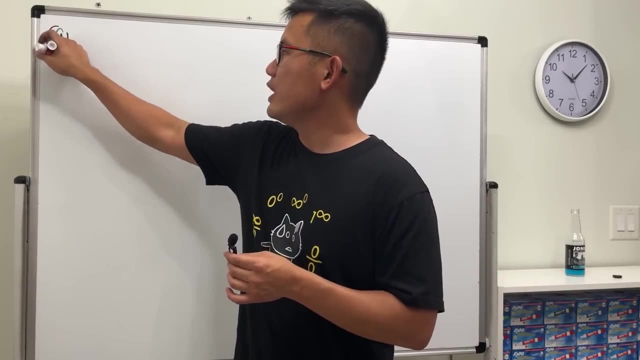 you know that you already, and I do have a very detailed explanation, and I do have a very detailed explanation, and I do have a very detailed explanation for remote some as well. so yeah, ladies for remote some as well. so yeah, ladies for remote some as well. so yeah, ladies and gentlemen, number 91 will come to a 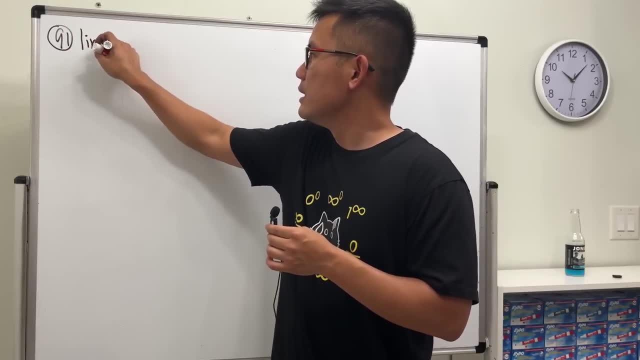 and gentlemen, number 91 will come to a and, gentlemen, number 91 will come to a. very, very long limit limit, as n goes to very, very long limit limit, as n goes to very, very long limit limit, as n goes to infinity. ready first one: 1 over n times. 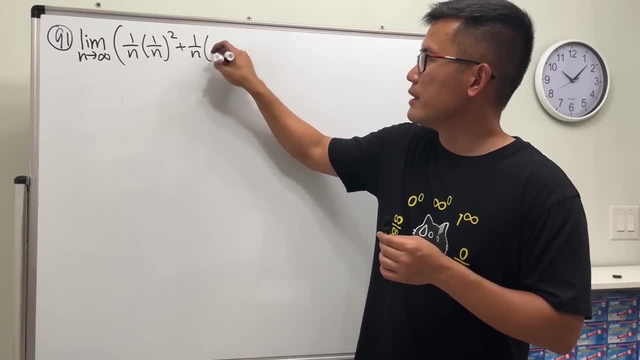 infinity ready. first one: 1 over n times. infinity ready. first one: 1 over n times 1 over n square. next one: 1 over n times 2. 1 over n square. next one: 1 over n times 2. 1 over n square. next one: 1 over n times 2 over n square. next one: 1 over n. 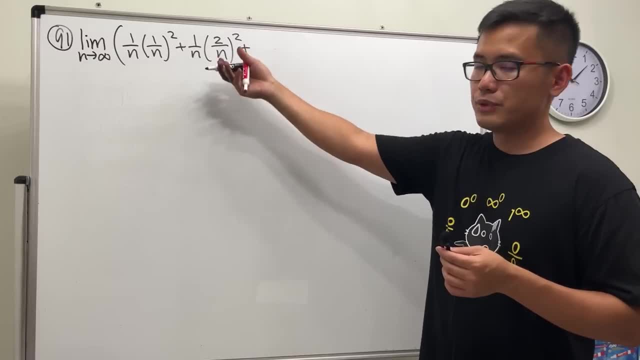 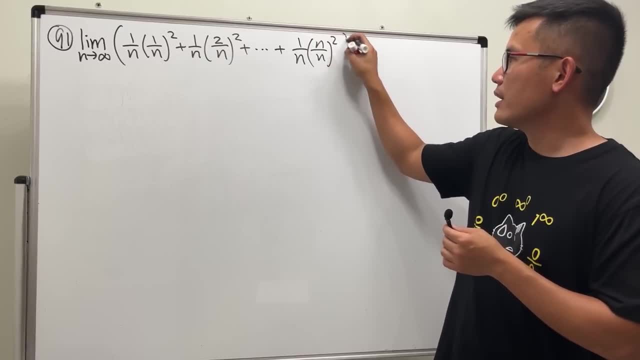 going to put on pasta data 1 over. going to put on pasta data 1 over n and over n square. alright. so there are a n and over n square alright. so there are a n and over n square alright. so there are a few ways that you can do it if you. 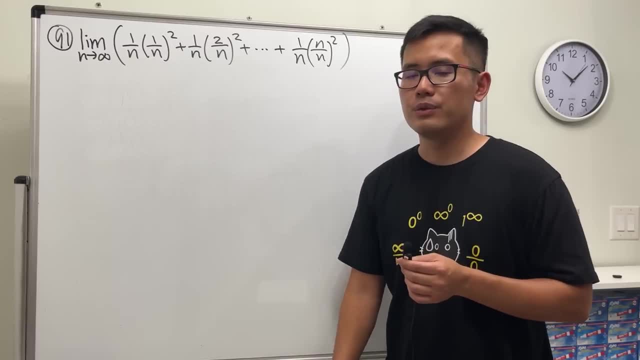 few ways that you can do it. if you few ways that you can do it, if you recognize what the region is, then you recognize what the region is, then you recognize what the region is, then you can come for that into integral, can come for that into integral. 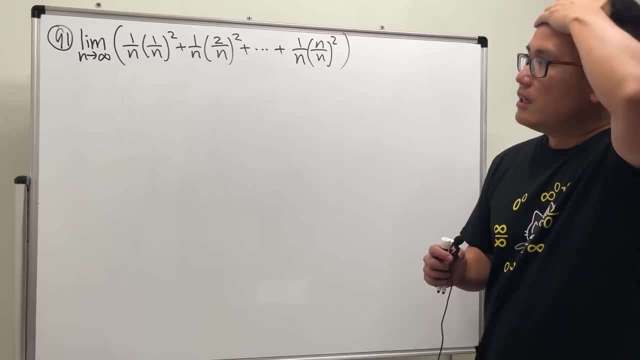 can come for that into integral question right away, so that's that. but question right away, so that's that. but question right away, so that's that. but what? this case? I want to show you guys what this case I want to show you guys what this case I want to show you guys at this one time, because this is 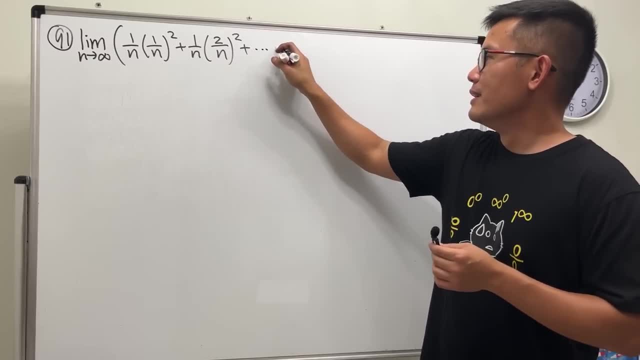 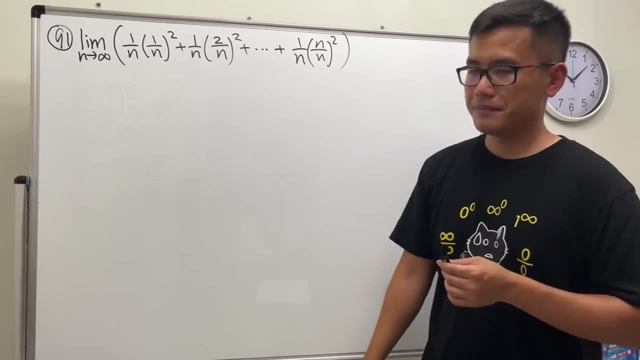 times 3 over n square. i'm not going to write that down, i'm just going to put on plus dot dot dot 1 over n n over n square. all right, so there are a few ways that you can do it if you recognize what the region is. 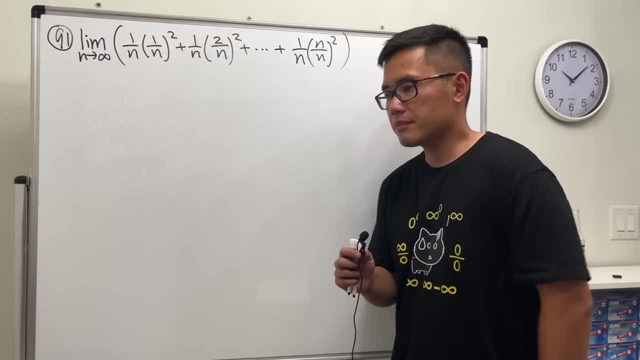 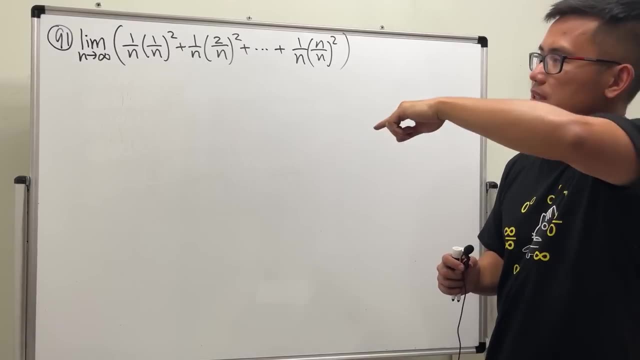 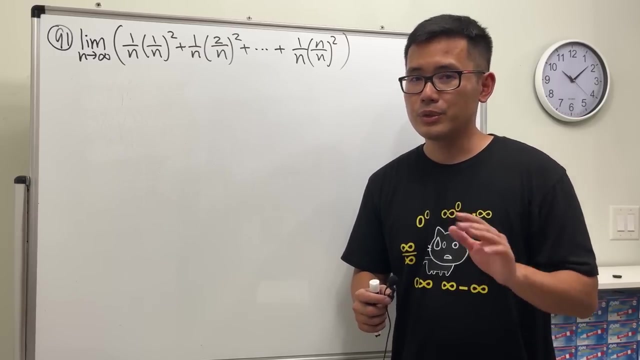 then you can convert that into, uh, integral question right away. so that's that. but for this case, i want to show you guys at this one time, because this is everybody's first definite integral, so i will show you guys how to do it, a very classic way, right? so 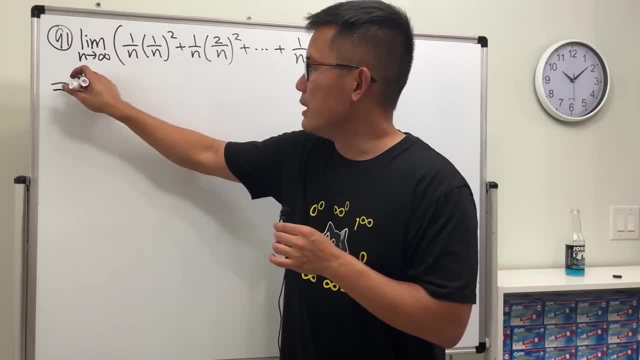 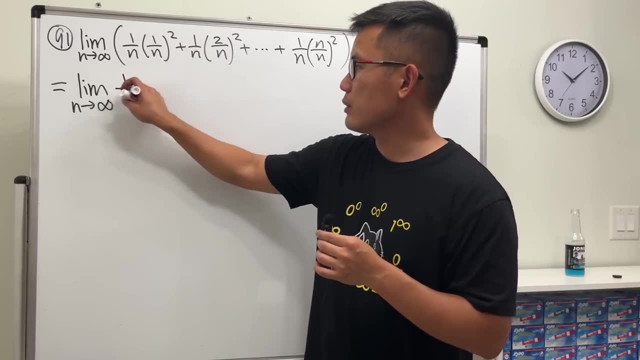 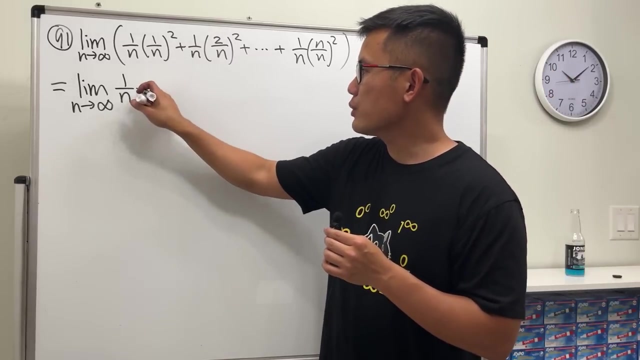 i'll show you. firstly, you keep the limit as n goes to infinity. and notice, everybody has the one over n, so i'm going to factor that out. in the meantime, though, n square, n square. everybody also has n square on the bottom as well, right, so i'm also going to 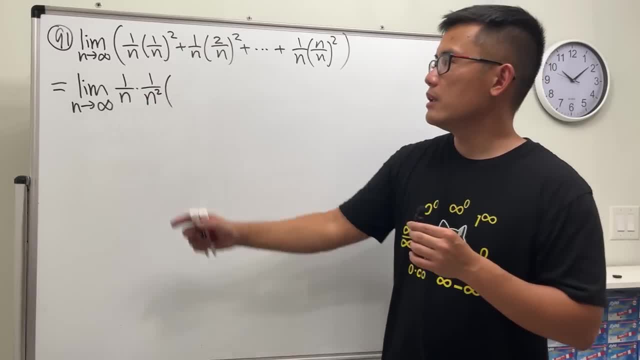 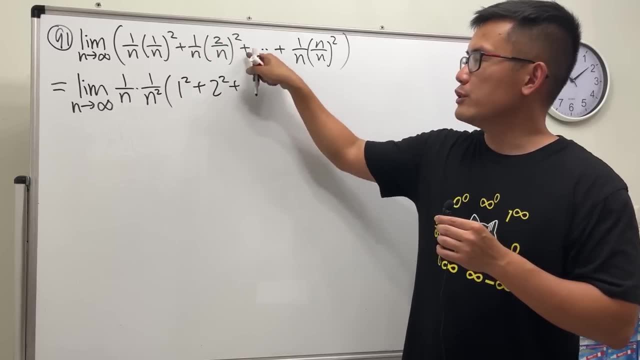 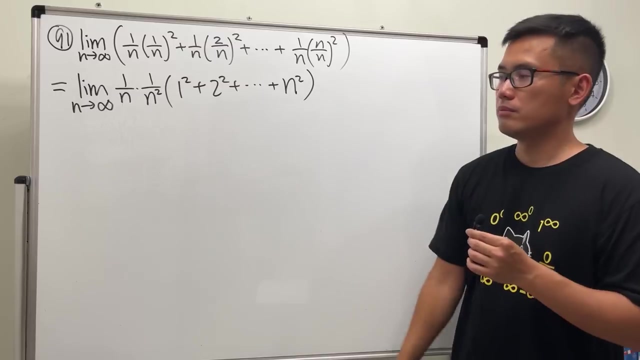 factor that out right here, and you will notice that this right here will just have one square left. next we will have two square left, and then three square left, and then so on, so on, so on, up to the very last part, which is n square, like so: 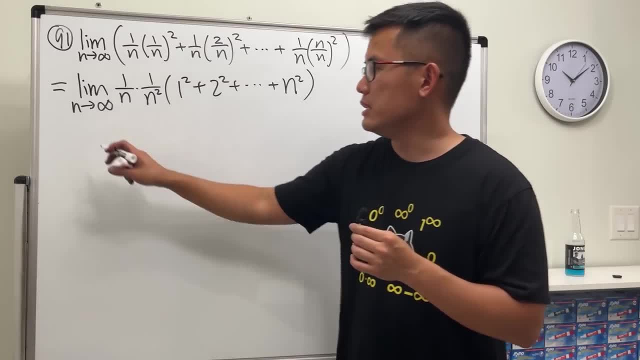 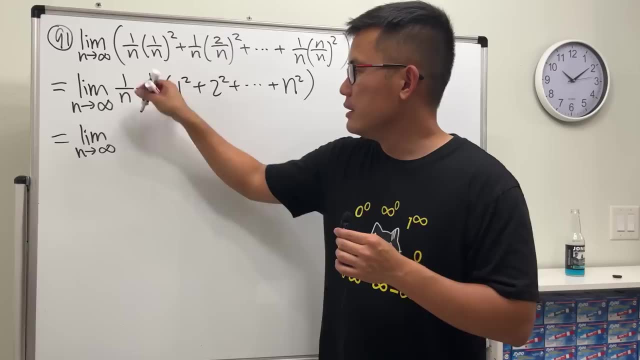 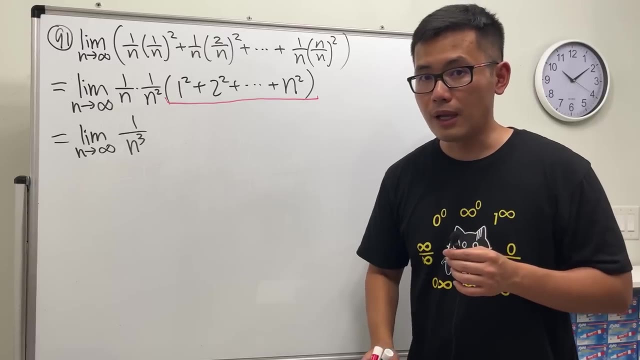 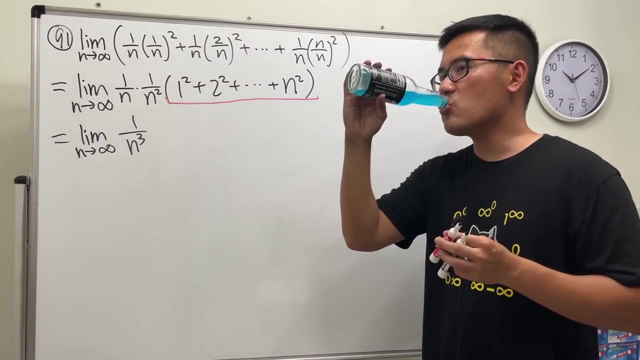 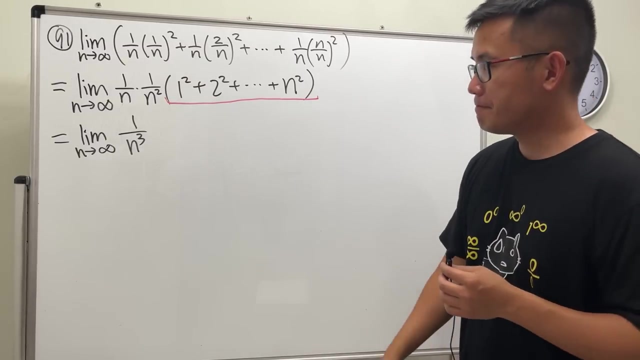 okay, then you are going to see, this is actually just very nice to be. n approaching infinity. this is one over n to the third power and all this. we have extremely nice formula. we have extremely nice formula. what is it? n times n plus one times two, n plus. 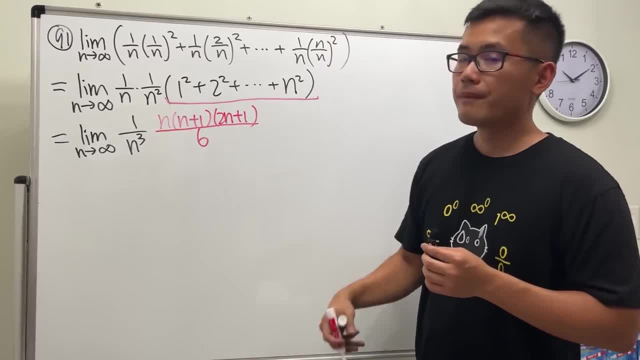 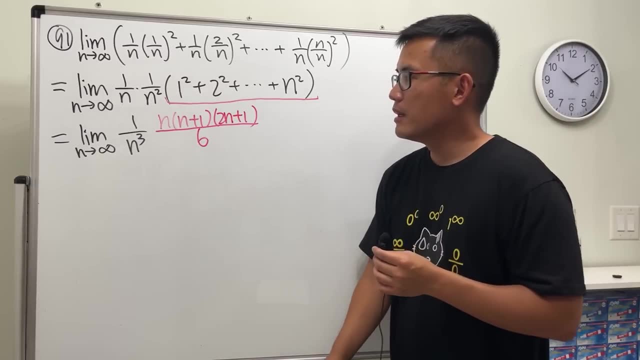 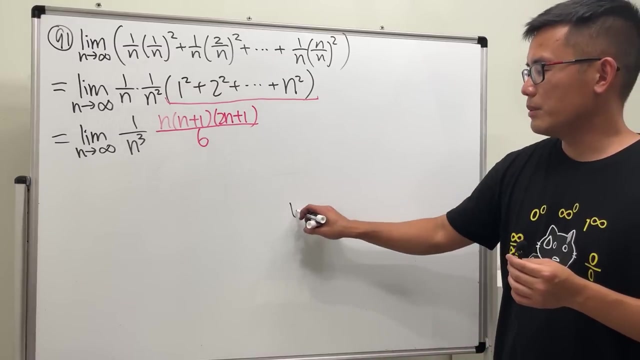 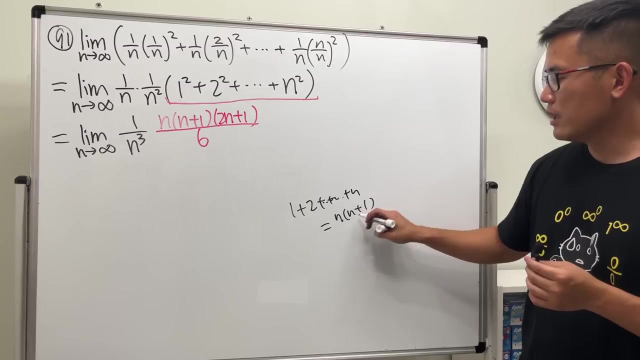 one all over six. check out my other video to see how we can prove this formula. alright, yeah, in fact, this is really cool because this formula actually contains one plus two plus three, plus up to n, because this right here is n times n plus one over two. 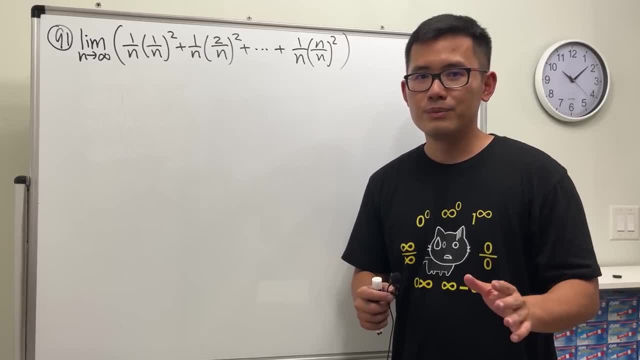 at this one time, because this is at this one time, because this is everybody's first definite integral. so I, everybody's first definite integral, so I, everybody's first definite integral, so I will show you guys how to do it a very. will show you guys how to do it a very. 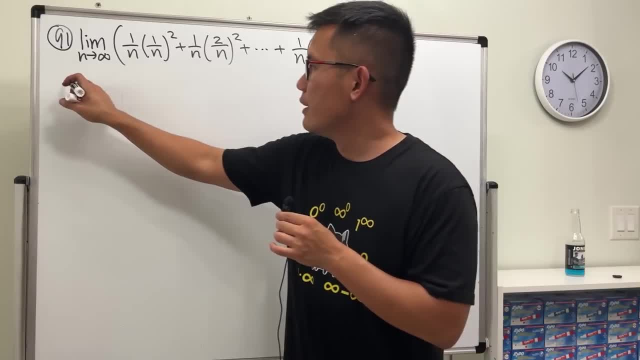 will show you, guys, how to do it- a very classic way. alright, so I'll show you classic way. alright, so I'll show you classic way. alright, so I'll show you. firstly, you keep the limit as n goes to. firstly, you keep the limit as n goes to. 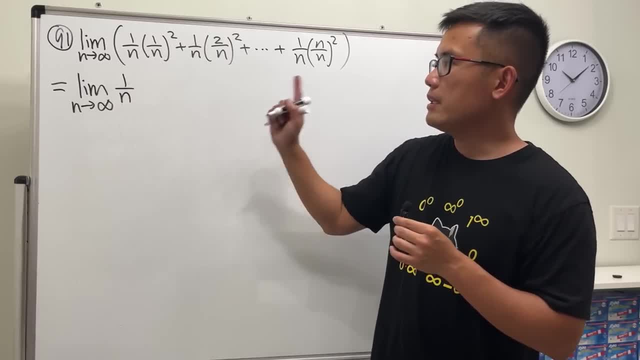 firstly, you keep the limit, as n goes to 1 over n. so I'm going to find out in the 1 over n, so I'm going to find out in the 1 over n, so I'm going to find out. in the meantime, though, and square and square. meantime, though, and square and square. meantime, though, and square and square, everybody also has n square on the. everybody also has n square on the. everybody also has n square on the bottom as well. right, so I'm also going bottom as well. right, so I'm also going. 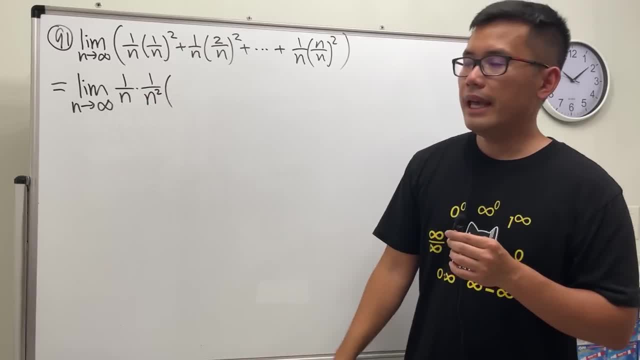 bottom as well, right? so I'm also going to factor that out right here, and you to factor that out right here, and you to factor that out right here, and you will notice that. this right here, we will notice that. this right here, we will notice that. this right here: we just have one square left. next we will: 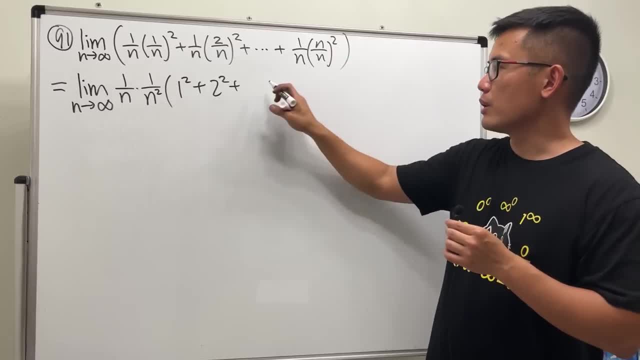 just have one square left. next, we will just have one square left. next we will have two square left and the street have two square left and the street have two square left and the street left, and so on, so on, so on, up to the very left, and so on, so on, so on, up to the very. 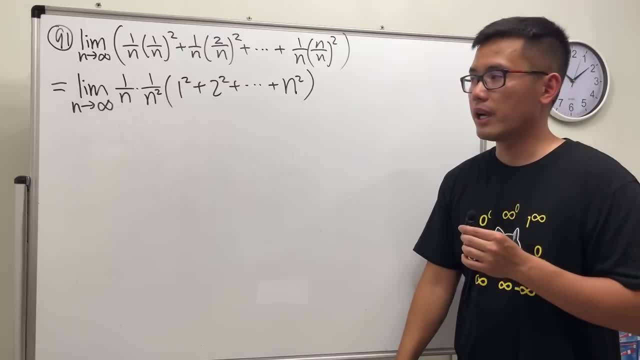 left, and so on, so on, so on, up to the very last part, which is n squared like so. last part which is n squared like so. last part which is n squared like so. okay, then you are going to see, this is okay. then you are going to see, this is. 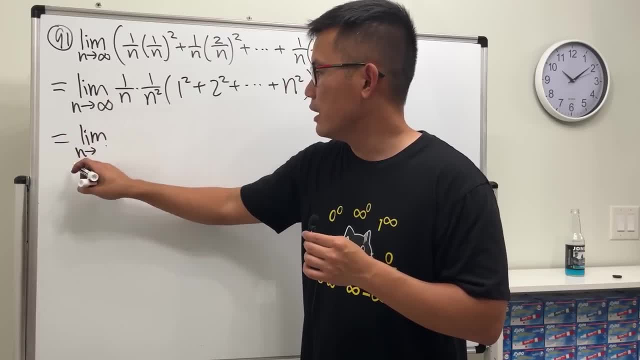 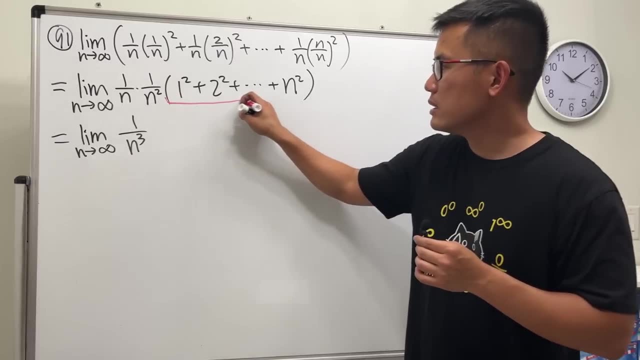 okay, then you are going to see, this is actually just very nice to be an, actually just very nice to be an, actually just very nice to be an approaching infinity. this is 1 over n to approaching infinity. this is 1 over n to approaching infinity. this is 1 over n to the third power, and all this we have. 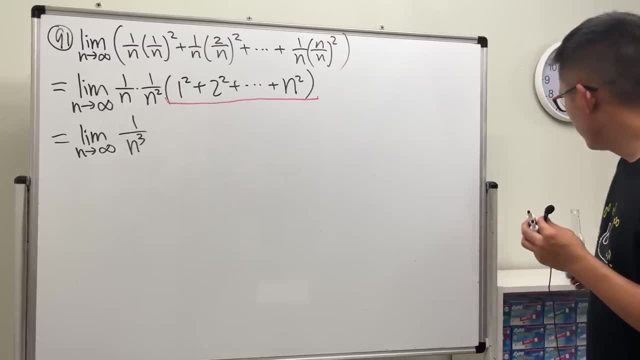 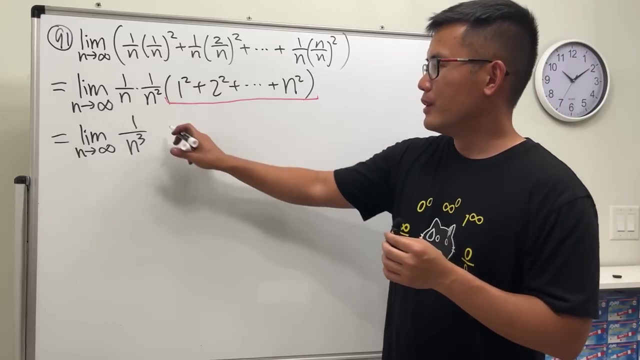 the third power and all this. we have the third power and all this. we have extremely nice formula and we have extremely nice formula and we have extremely nice formula and we have extremely nice formula. what is it ready n times? what is it ready n times? what is it ready n times n plus 1? times 2n plus 1? 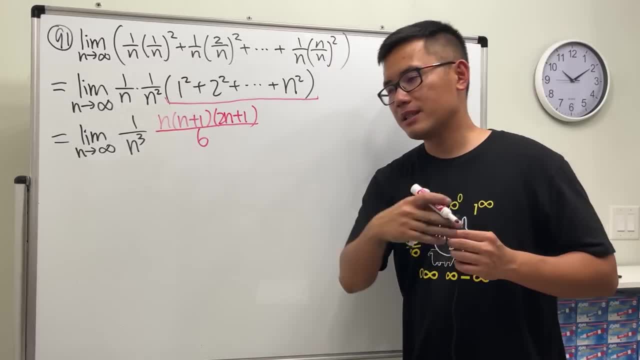 n plus 1 times 2n plus 1. n plus 1 times 2n plus 1- all over six, all over six. all over six. check out my other video to see how we check out my other video, to see how we check out my other video, to see how we can prove this formula. 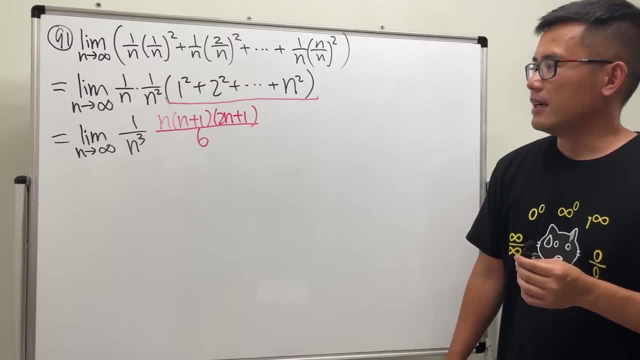 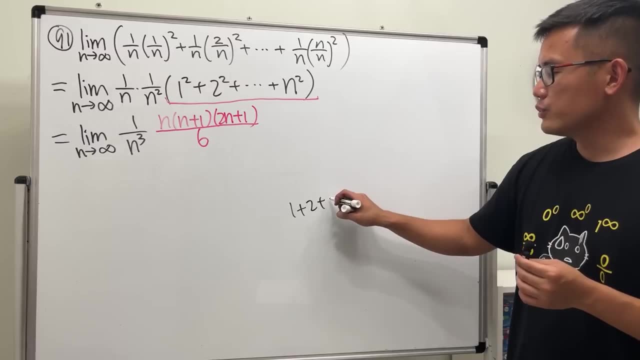 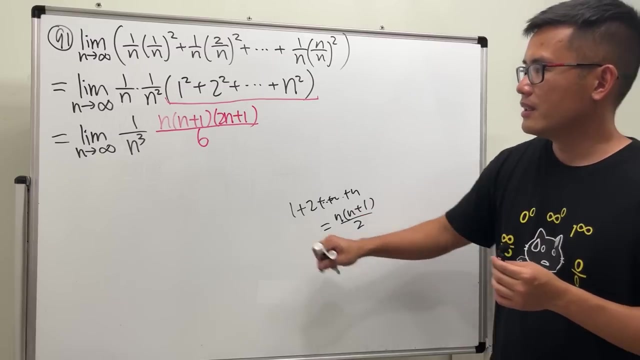 can prove this formula. can prove this formula, all right. yeah, in fact, this is really cool because this formula actually contains one plus two plus three plus up to n, because this right here is n times n plus one over two, so we have the n times n plus one. break this down as two times three. 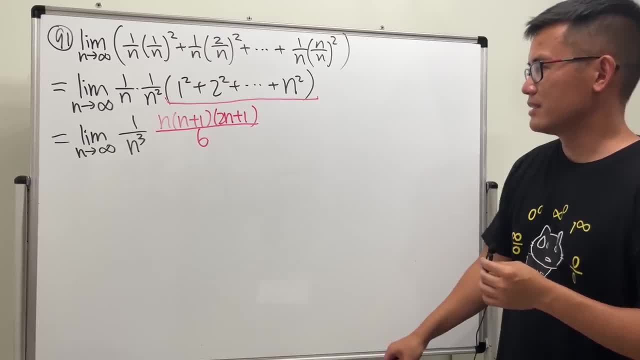 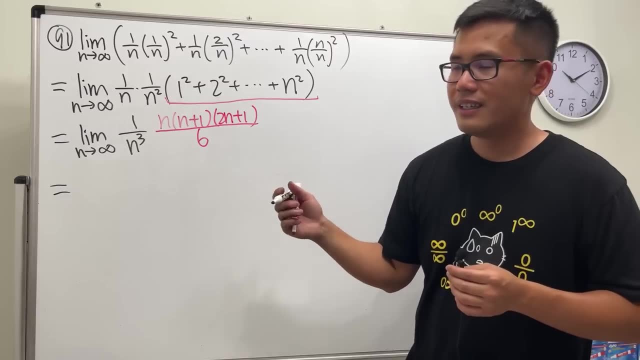 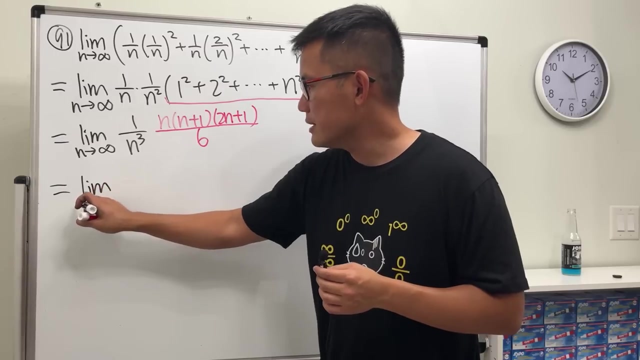 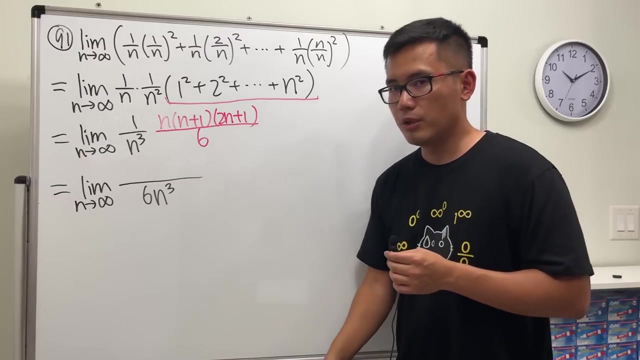 yeah, but that's a discussion for another video. anyway, does this look familiar? you should the limit as something to the to approach infinity, right? so this is the limit as n goes to infinity. on the bottom we have six n cube on the top. just for fun, i'm going to multiply out for you guys. here we have n square. 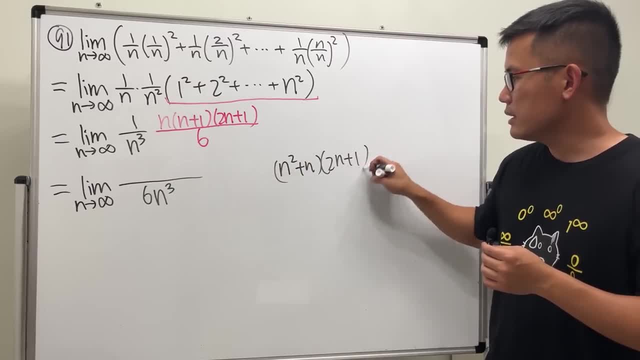 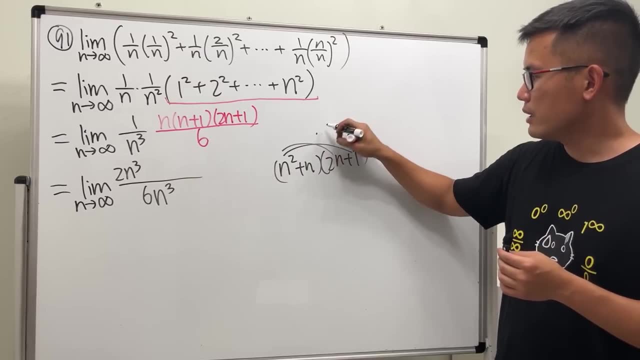 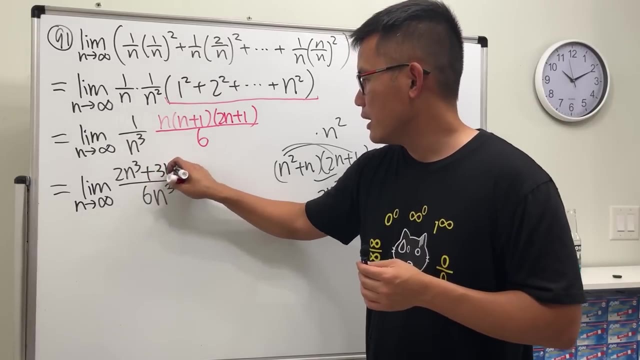 plus n, and then we multiply 2n plus 1. so this right here is 2n to the third power, and then n square, and then 2n squared. yes, together is 3n square. and lastly, we have n? right, you really don't have to multiply. 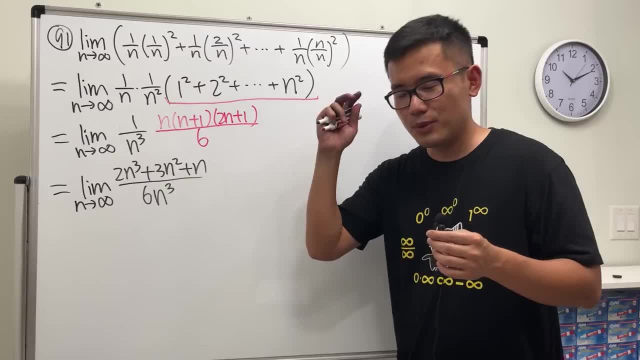 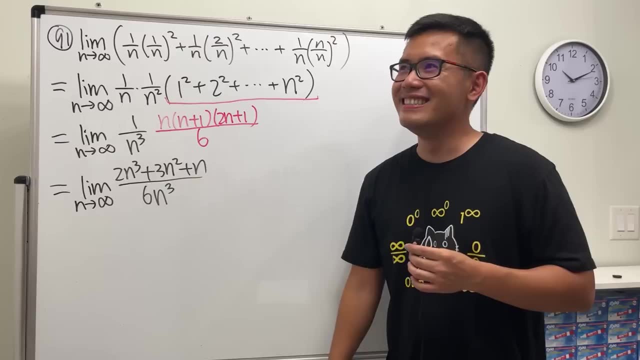 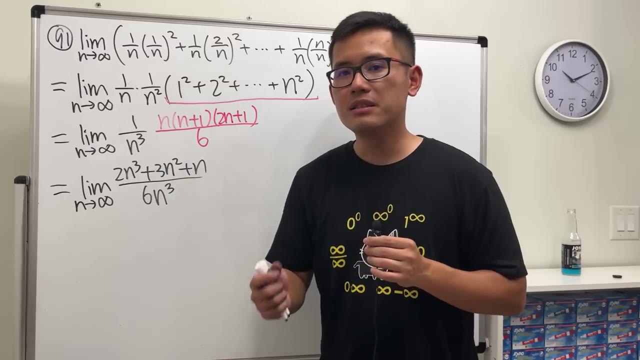 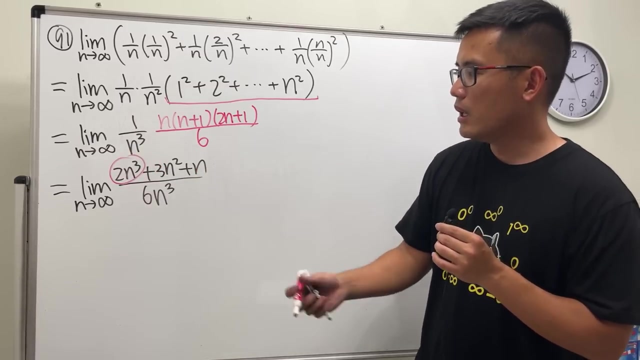 out everything but number. question number number 21. my soul is loading, leaving my body. limit is n approaching infinity. this is everybody's favorite calculus question. on the top, we care about two to the. so we care about two. n to the third power. on the bottom, we also have the same thing. n to the third power. they cancel out. reduce two and six. we. 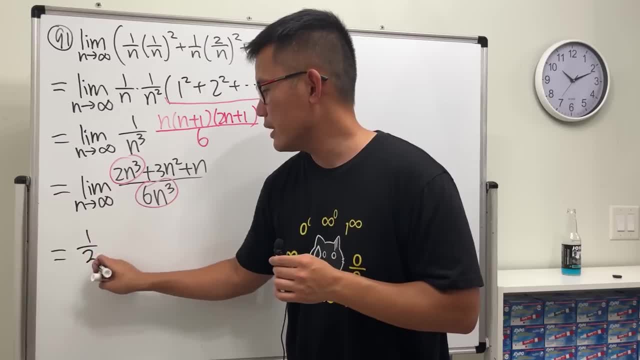 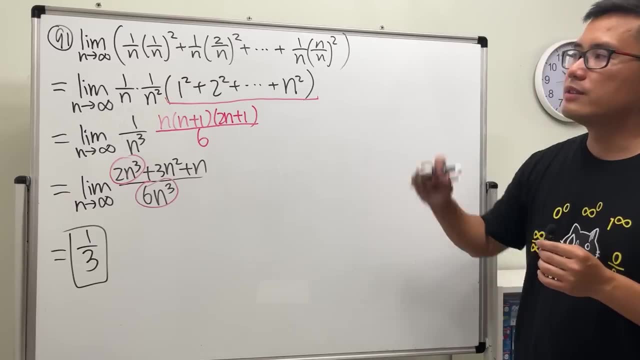 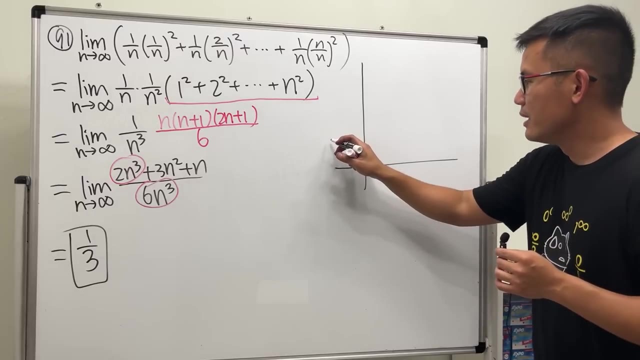 get one third. hey, the answer is just one third. very, very nice, very, very nice. all right, now it's about time to tell you guys what this represents. this, as i said, is everybody's first integral question and it's just going to be the area under x square. 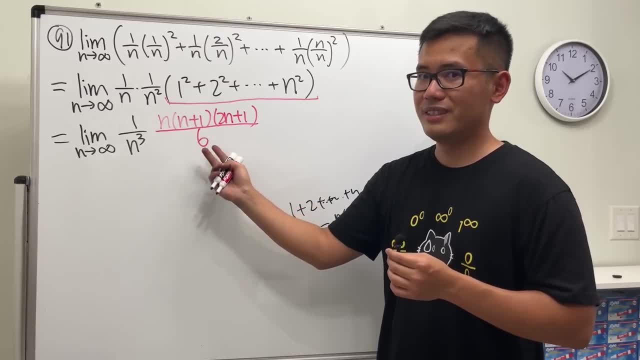 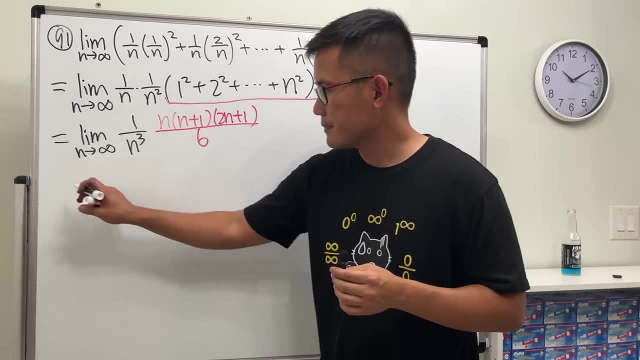 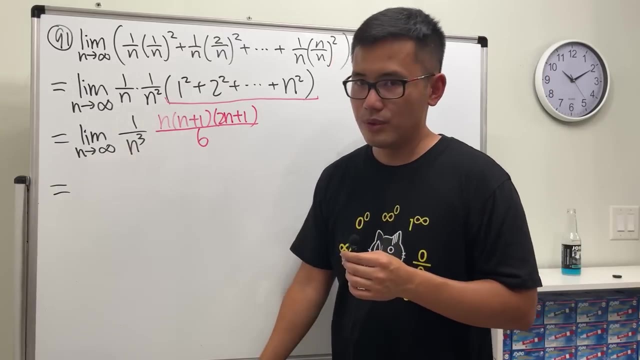 so we have the n times n plus one. break this down as two times three. yeah, but that's a discussion for another video. anyway, does this look familiar? you should. the limit is something to the to approach infinity, right, so this is the limit as n goes to infinity on the. 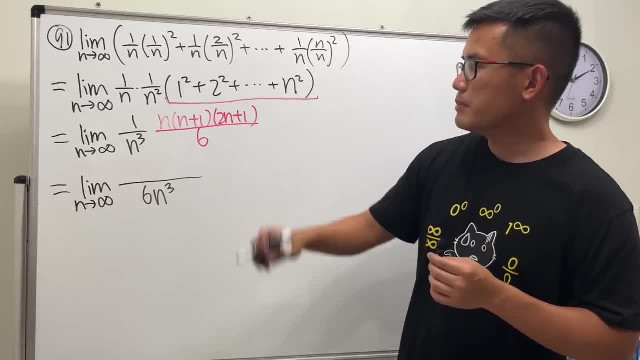 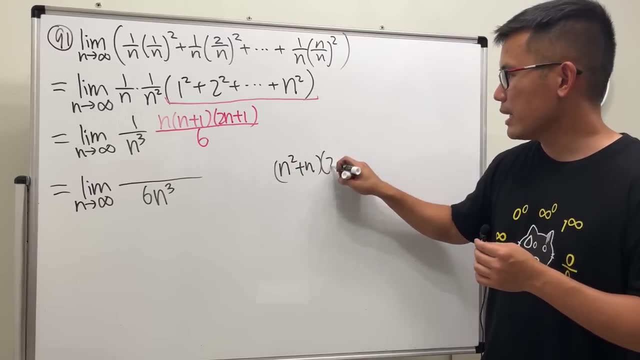 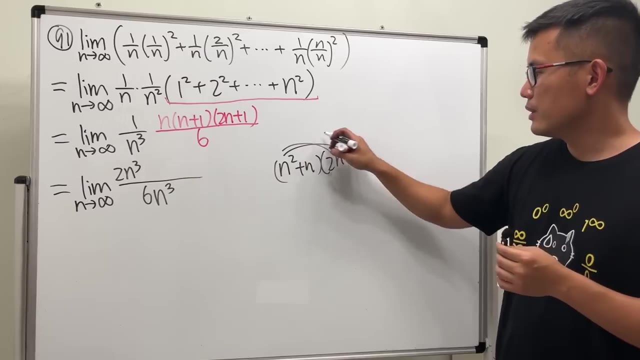 bottom we have six n cube on the top. just for fun i'm going to multiply out for you guys. here we have n square plus n, and then we multiply two n plus one. so this right here is two n to the third power and then n square. 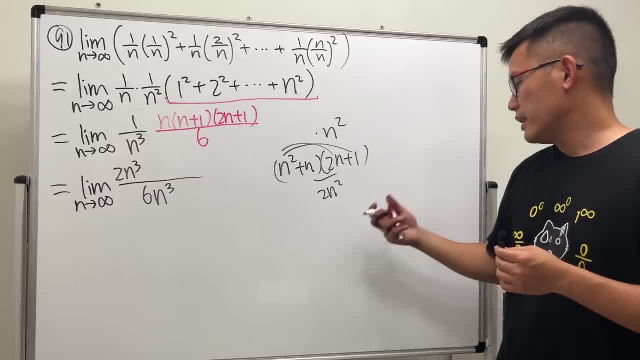 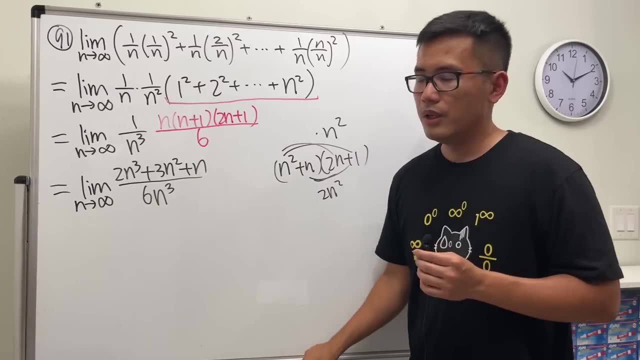 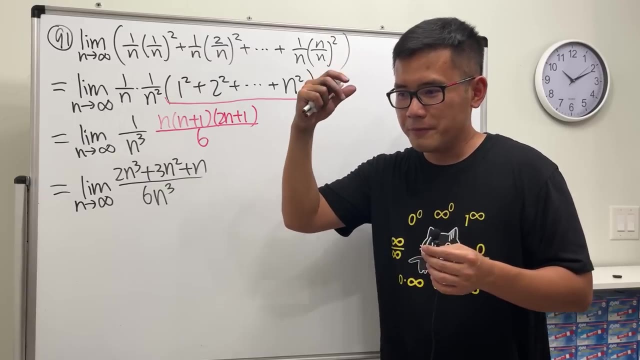 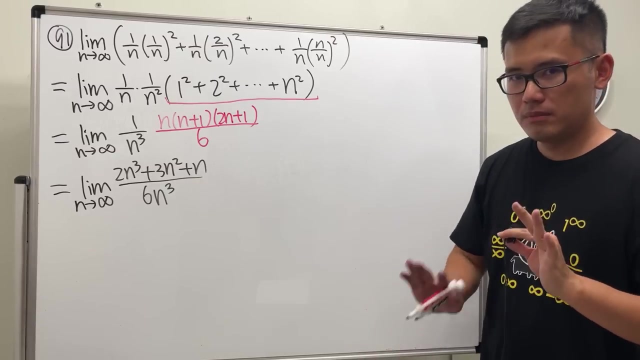 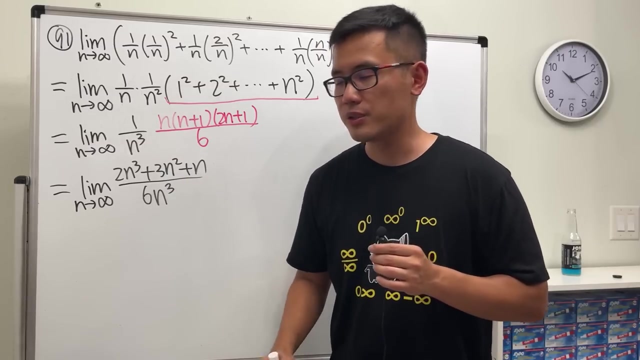 and then two n square. yes, together is three n square. and lastly we have n. you really don't have to multiply out everything but number. question. number number 21: my soul is loading, leaping. my body limit is n approaching infinity. this is everybody's favorite calculus question. 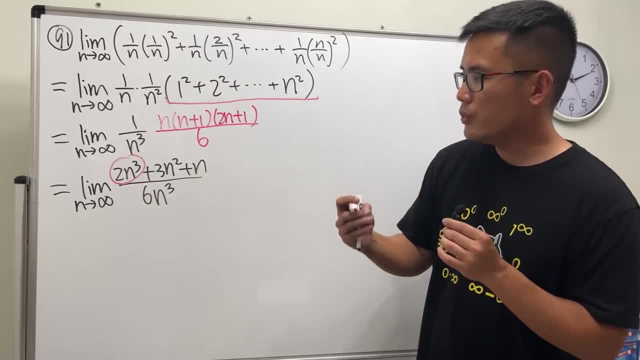 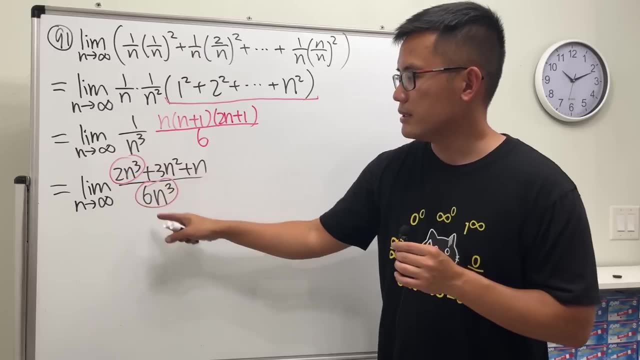 on the top, we care about two to the sorry, we care about two. n to the third power on the bottom, we also have the same thing. n to the third power they cancel out. reduce two and six, we get one third. hey, the answer is just one third. very. 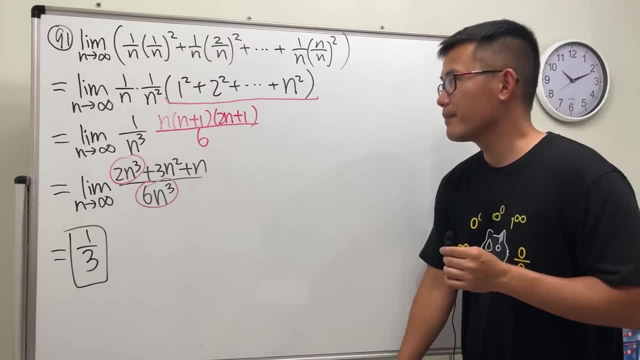 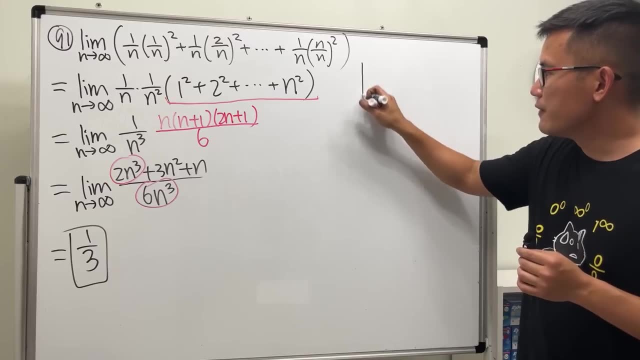 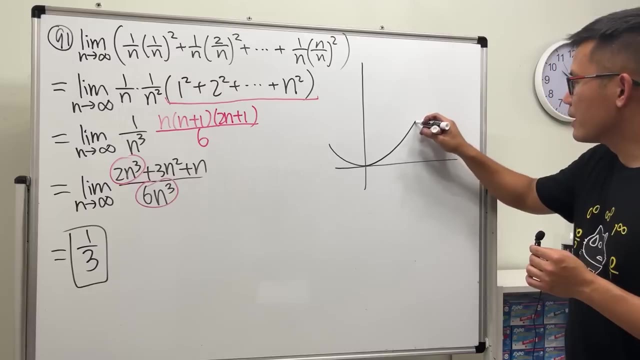 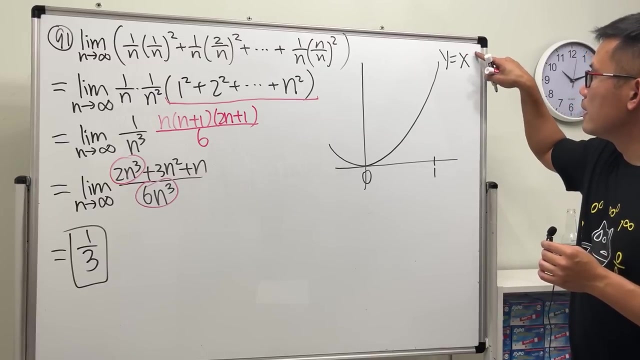 very nice, very, very nice. all right, now it's about time to tell you guys what this represents. this, as i said, is everybody's first integral question, and it's just going to be the area under x square from zero to one. how well, i'm going to. 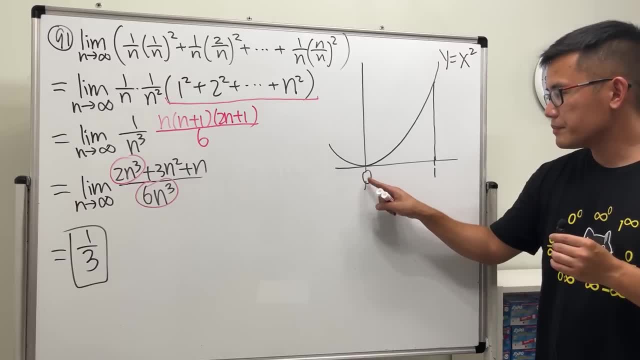 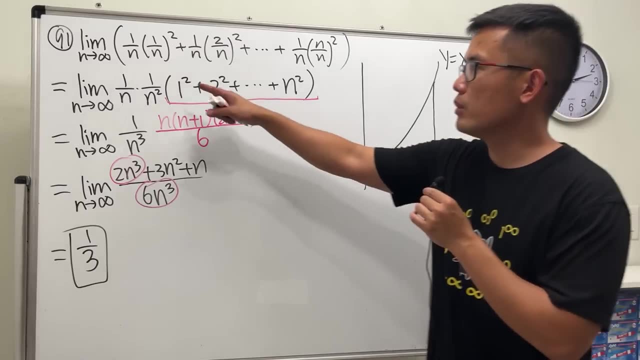 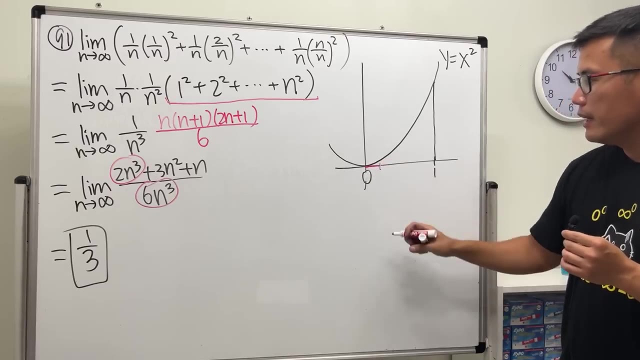 show you, don't worry, when we have zero to one. the idea is that we are going to cut this into n equal width rectangles. that's why we have all the one over n. so just imagine we come to an equal piece rectangles. so this is the first piece and i'm going to 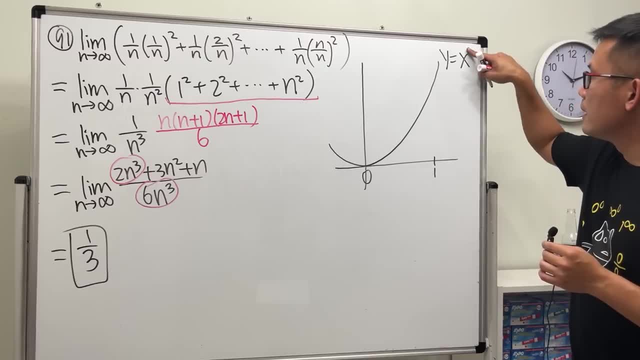 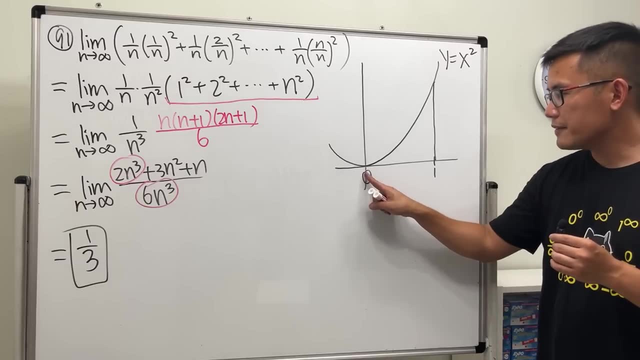 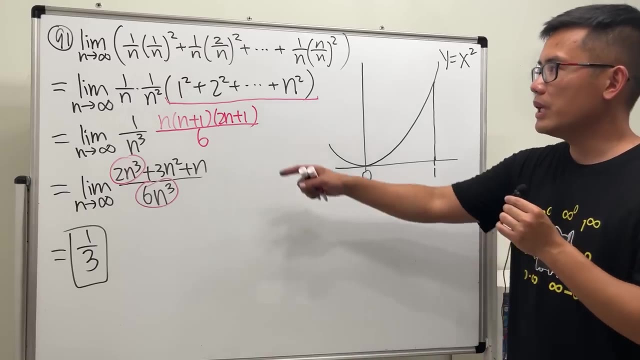 from 0 to 1. how well i'm going to show you, don't worry. when we have 0 to 1, the idea is that we are going to cut this into n equal widths rectangles. that's why we have all the 1 over n, so just. 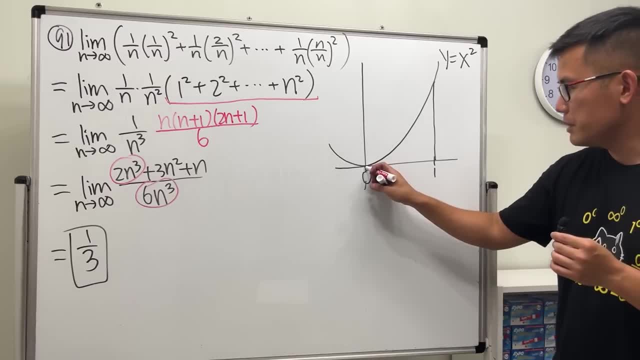 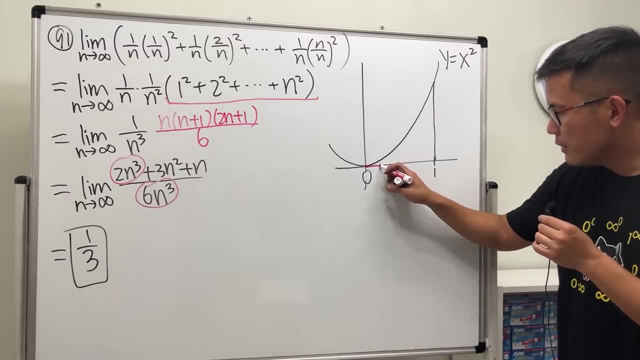 imagine we come to an equal piece rectangles. so this is the first piece and i'm going to use the right end point to construct the rectangle, meaning that, use this x value, go up, hit the curve, and then we are going to just construct our rectangle right here. 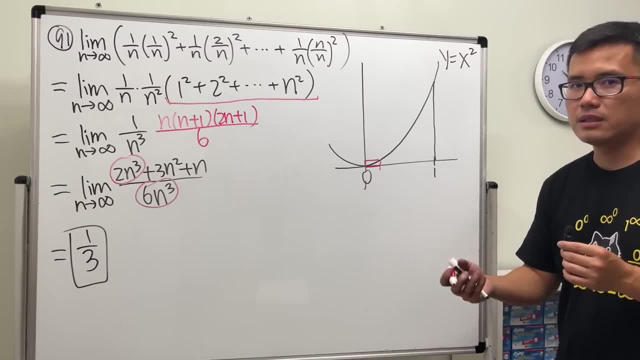 and because we have n rectangles, just imagine a 10. then in this case will be like 1 over 10, right, but against n. so this right here is 1 over n. what's the height of this rectangle? it's just a y value. we use this x for you: 1 over n. we put it here and we get. 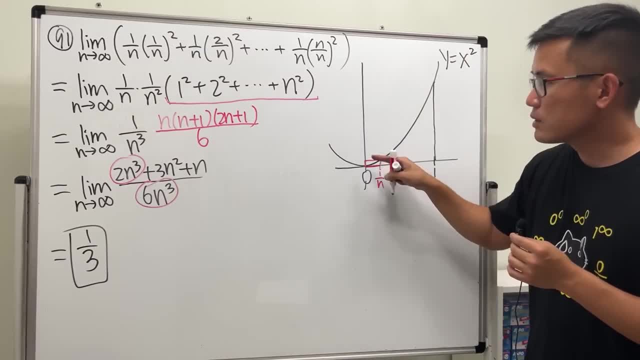 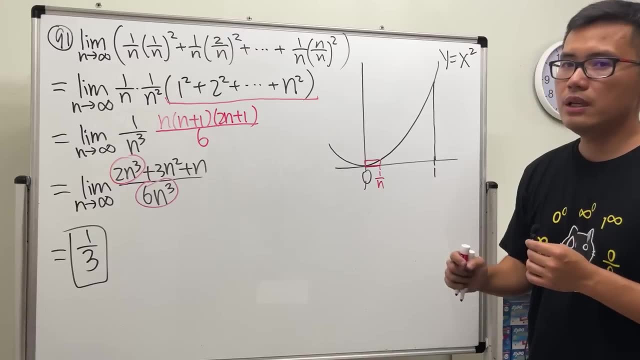 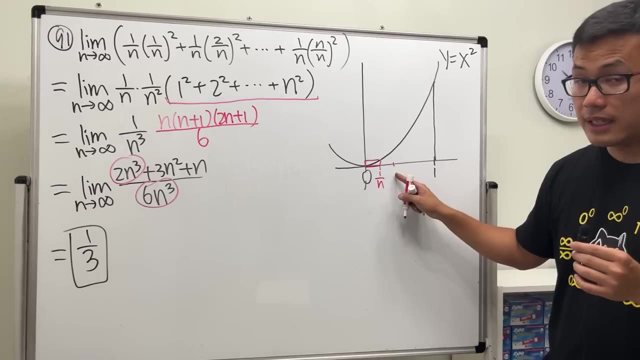 1 over n square. so this height is 1 over n square times. the base is 1 over n. so this right here is the area of the first rectangle, next where we have this rectangle here, but it go up by another 1 over n. so this x for you is 2 over n. so go up, hit the curve. 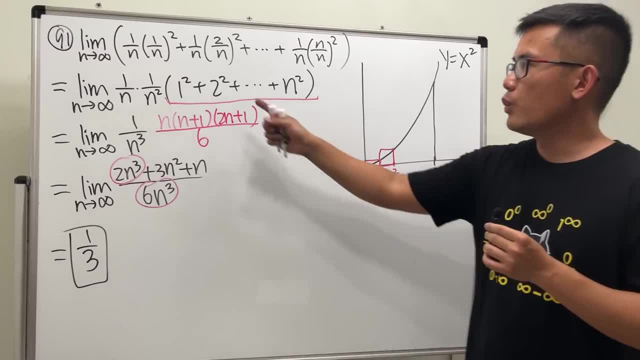 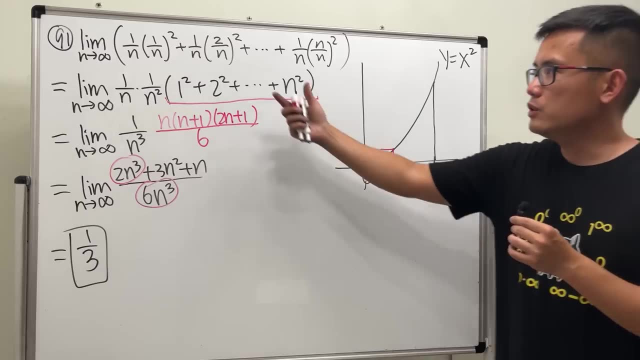 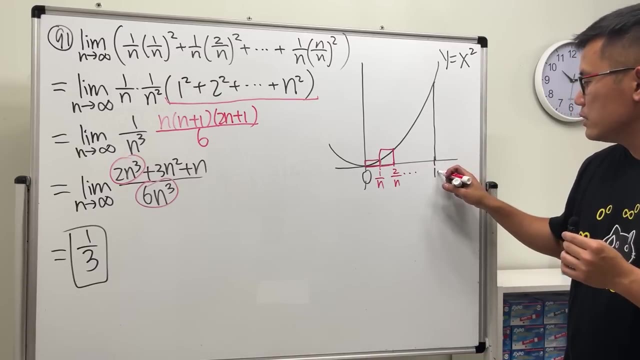 and then construct the rectangle. the width is still 1 over n, though, but the height? we put 2 over n in to the x, so we get 2 over n square. so this right here represents the area of the second rectangle. so on, so on, so on, and the very last one is 1, which is just the same as n over n. we go up. 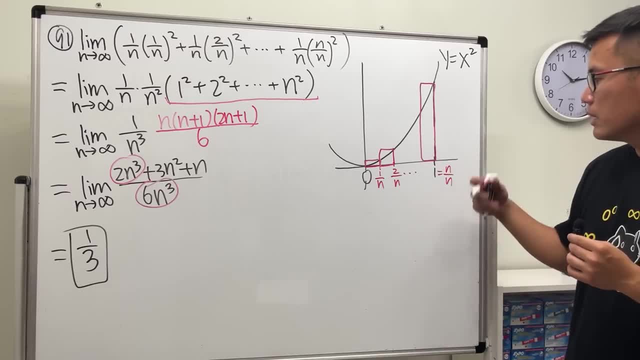 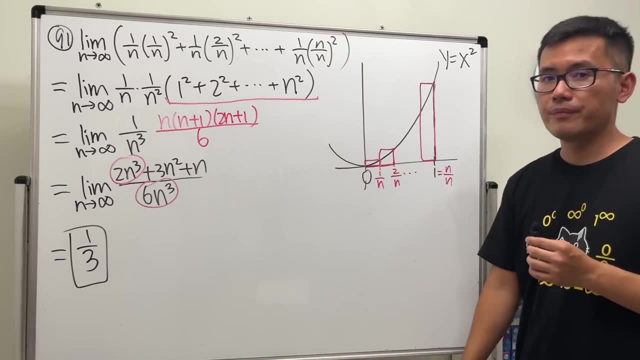 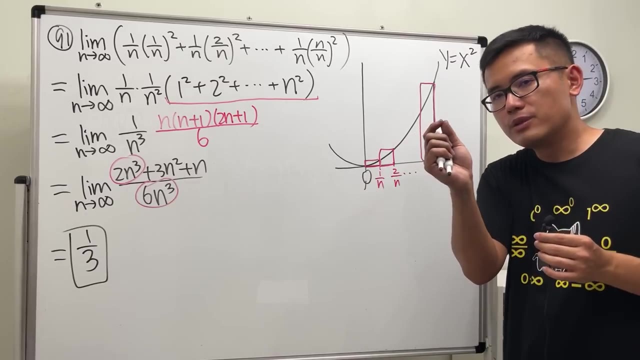 hit the curve, and then we construct our rectangle, yeah, which is still 1 over n, the highest, n over n square, the area of the last vertical, as we have n, approaches infinity. each rectangle is going to be so, so, so, so so thin, like infinitesimal small. 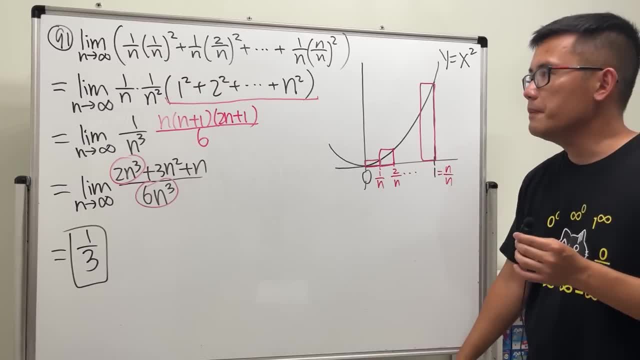 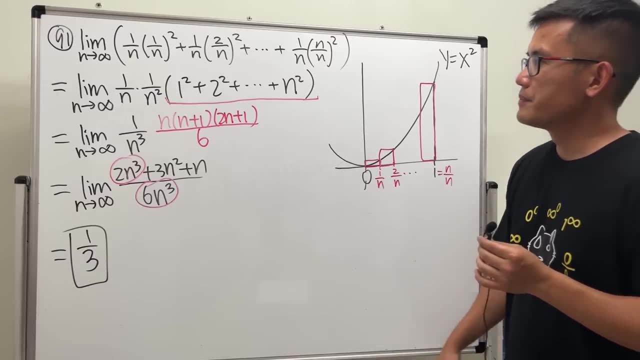 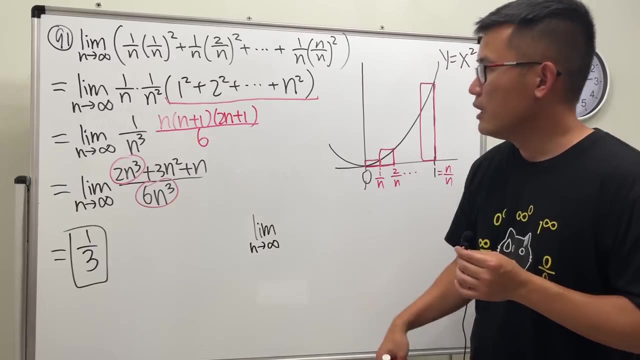 yeah, so you can actually get the area. okay, all right, so that's cool. but i want to show you guys what's cooler. check this out. this right here is just a way to say we have the limit as n goes to infinity, and then you see that. 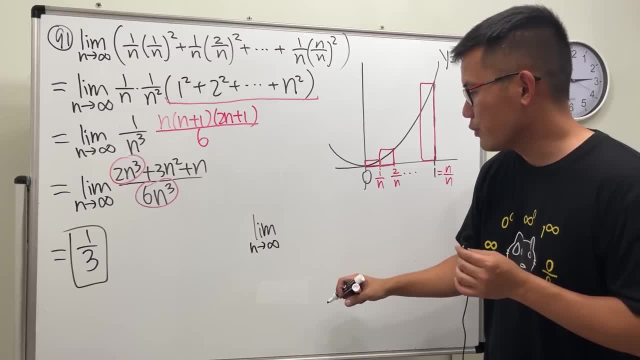 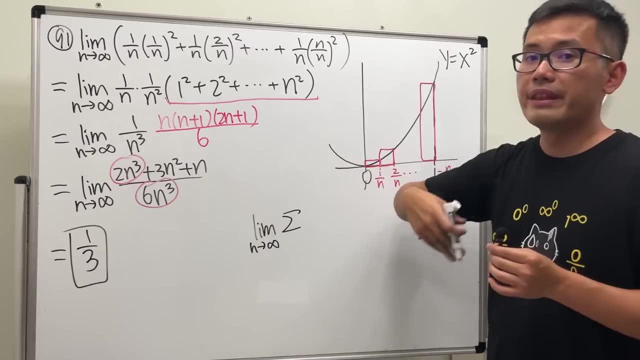 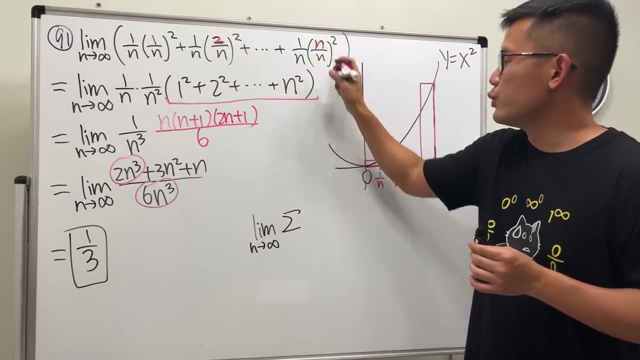 we have all the addition, which is the summation, which we can use sigma for it. we can write it as sigma like this: and then you see, we have the one, two, three, up to n. they changes right. they change right. so that's where we need to use the running index. we will. 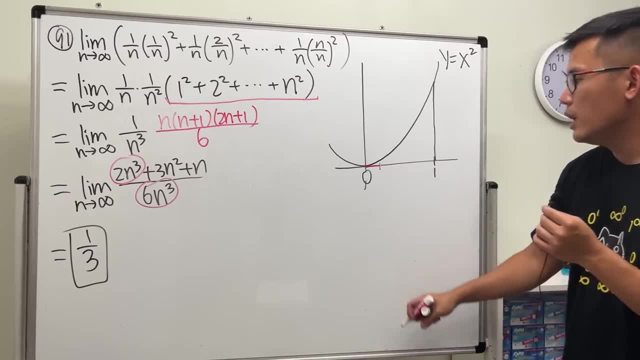 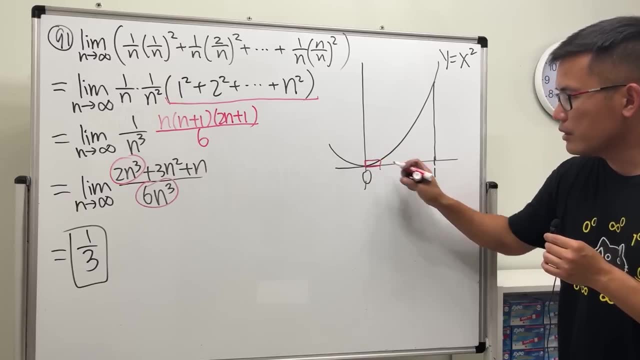 use the right end point to construct the rectangle, meaning that use this x value, go up, hit the curve, and then we are going to just construct our rectangle right here. and because we have n rectangles, just imagine a ten. then in this case would be like one over ten, right but against n. 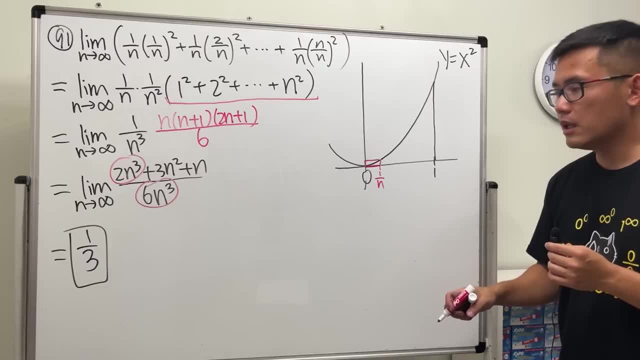 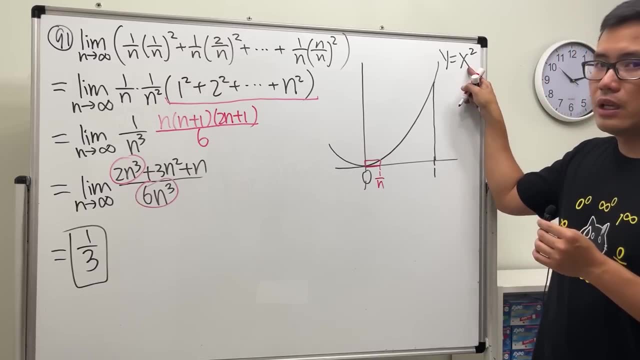 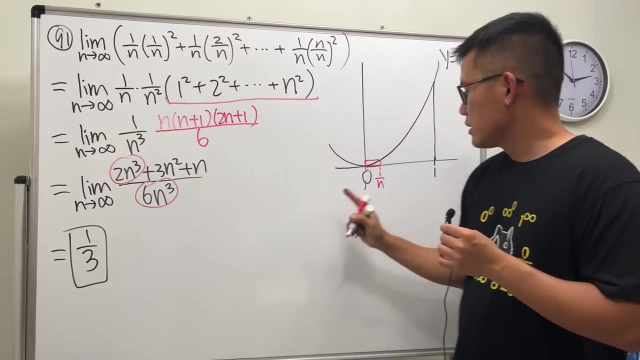 so this right here is one over n. what's the height of this rectangle? it's just a y value. we use this x value, one over n, we put it here and we get one over n square. so this height is one over n square times. the base is one over n. so this right. 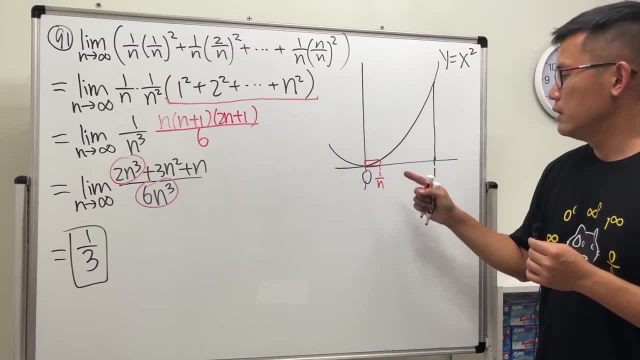 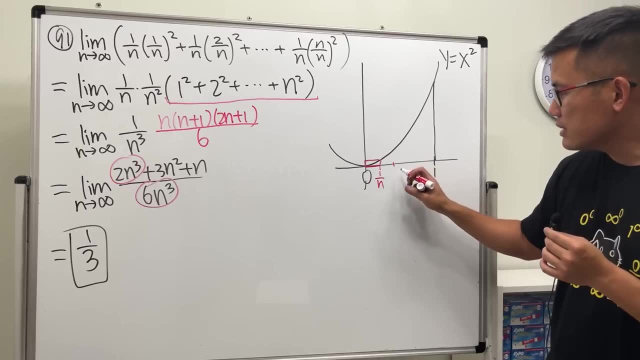 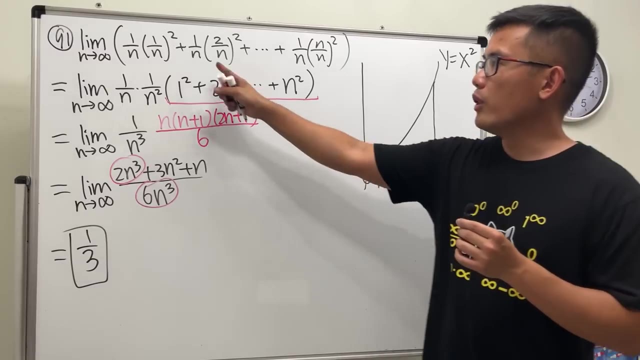 here is the area of the first rectangle, next where we have this rectangle here, but it go up by another one over n. so this x value is two over n. so go up, hit the curve and then construct the rectangle. the width is still one over n, though, but the height we put 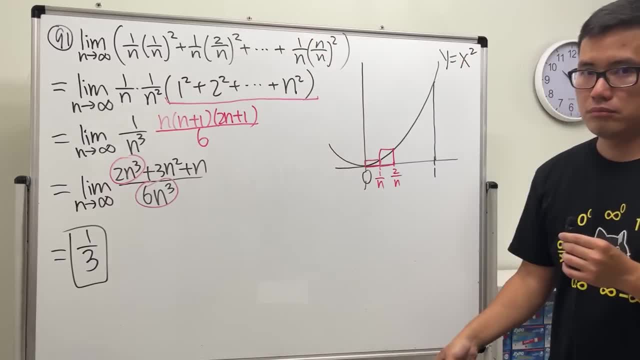 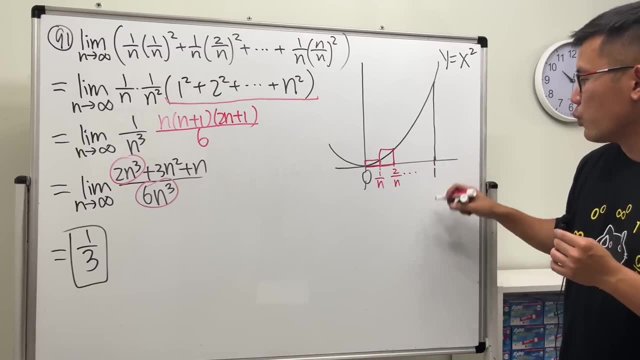 two over n into the x. so we get two over n square. so this right here represents the area of the second rectangle. so on, so on, so on, and the very last one is one which is just the same as n over n. we go up, hit the curve. 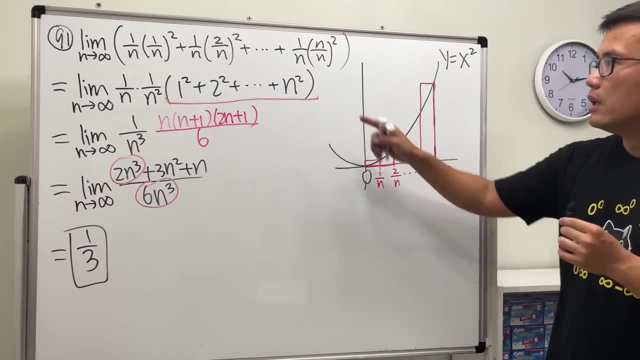 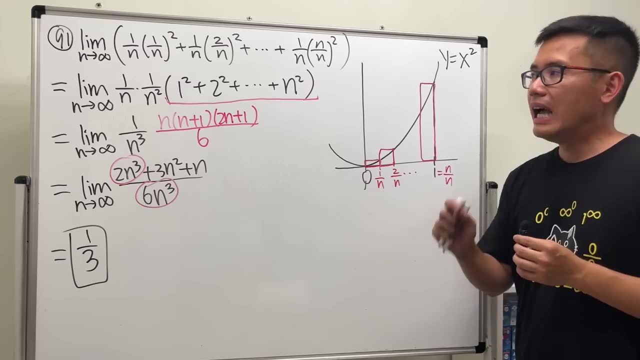 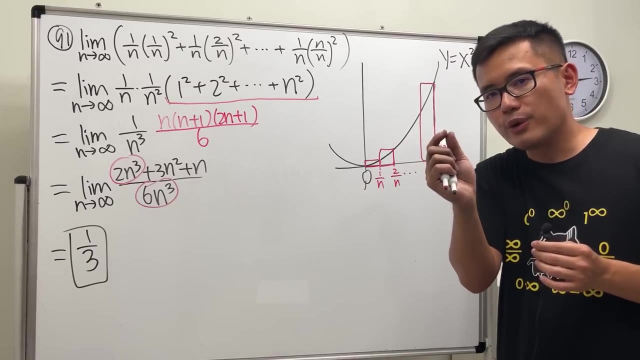 and then we construct our rectangle. yeah, width is still one over n, the height is n over n. square. the area of the last rectangle, as we have n, approaches infinity. each rectangle is going to be so, so, so, so, so thin, like infinitesimal small. yeah, so you can actually get the area. 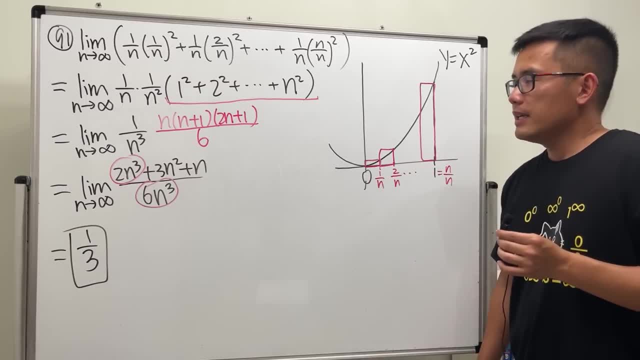 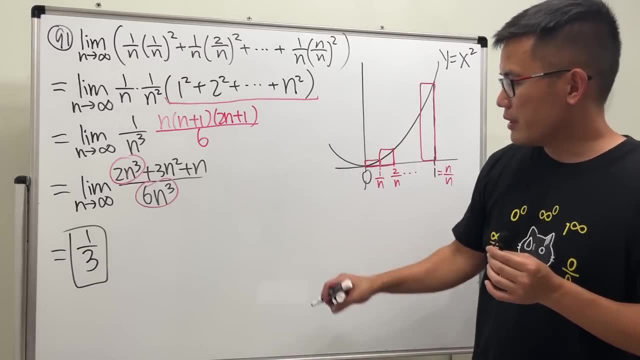 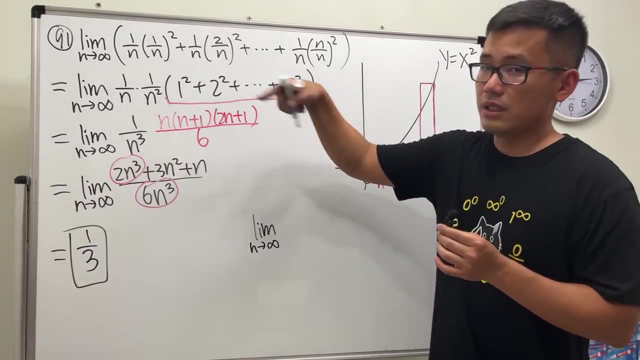 okay, all right. so that's cool, but i want to show you, guys, what's cool. check this out. this right here is just a way to say we have the limit as n goes to infinity, and then you see that we have all the addition, which is the summation which we can use: sigma. 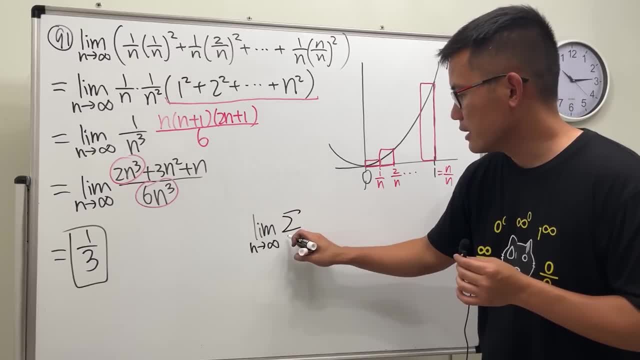 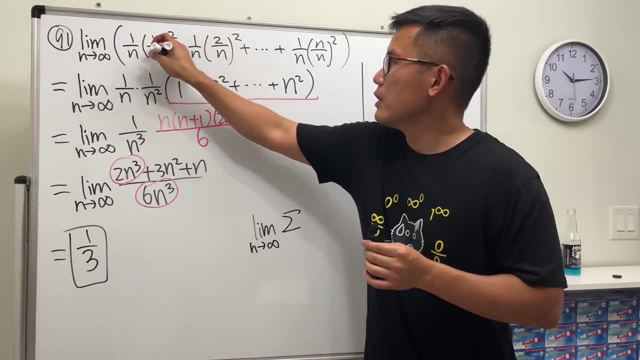 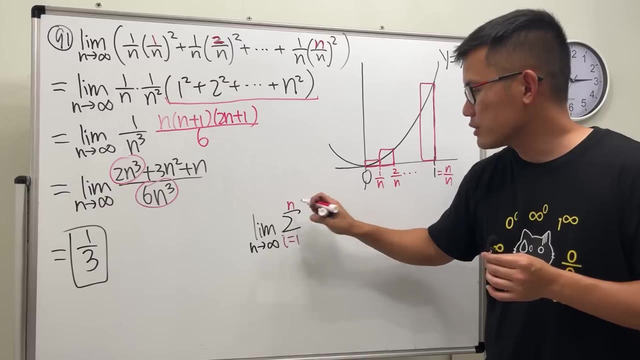 for it. we can write it as sigma, like this, and then you see, we have the one, two, three, up to n. they changes right, they change right. so that's where we need to use the running index. we will say: i just the running index, i goes from one to n. 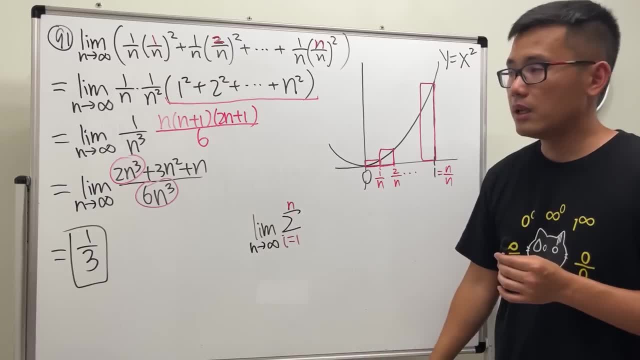 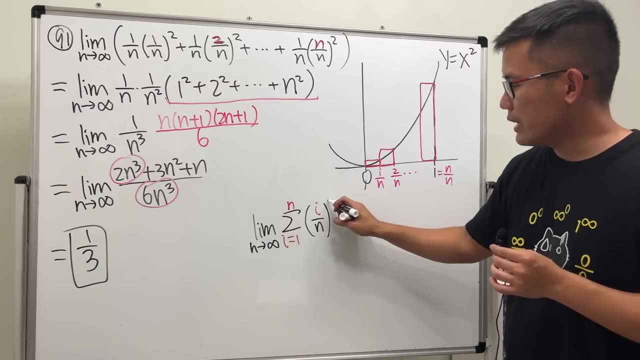 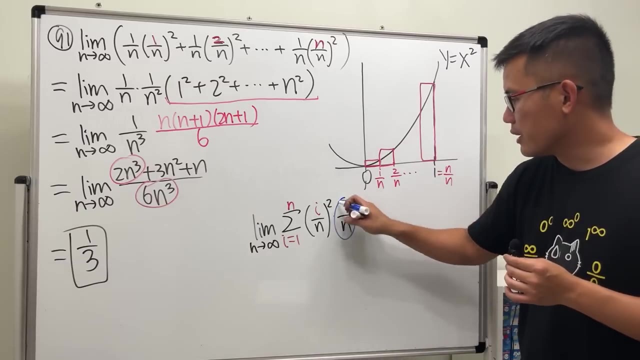 say i just the running index. i goes from one to n inside. here we have i over n, yeah, and then we square that and then we multiply by one over and i just put one over at the end. this right here is the width, aka delta x, delta x. another way to look at it is: 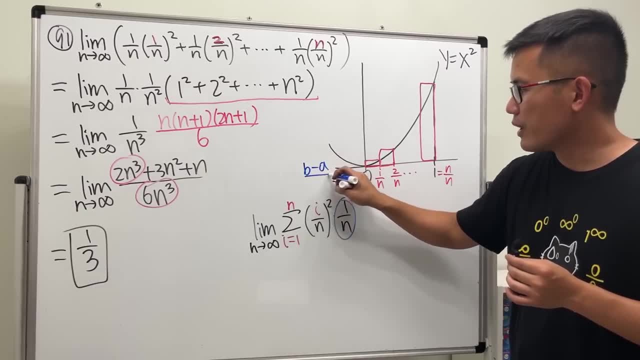 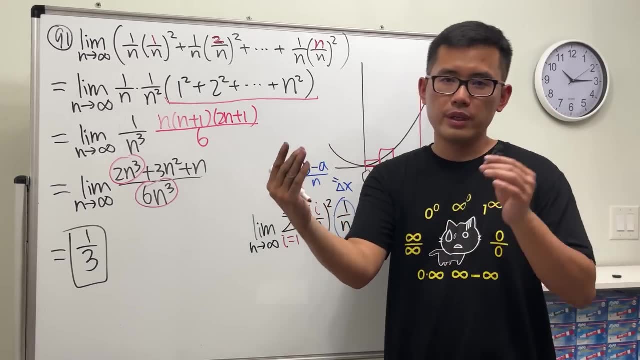 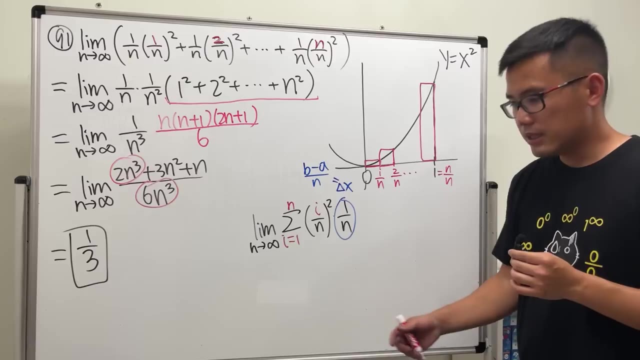 from where to where, and we write it as b minus a over n. so the range, right, it's only one unit away. if we start with 0, we end up with 1.. if we start with 17, we end up at 18.. so that's the structure. and guess what? if you know the structure of this, we can change this to a. 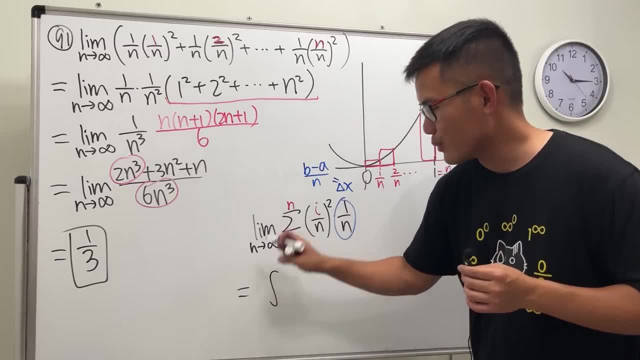 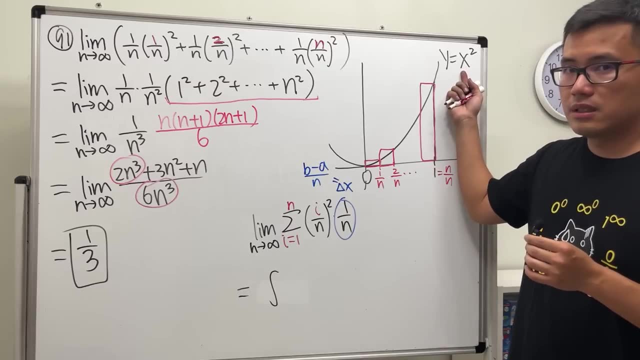 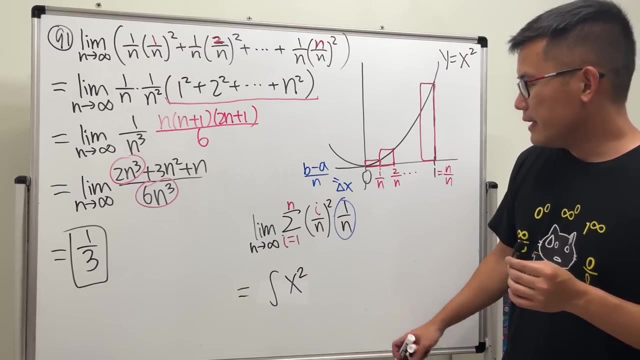 super version, that is the so-called integral. what's the function? you see, the input is i over n. that's what we talk about. we enter all this into the x, so that's the function. so the function in this case is x squared. yeah, and then you can actually look at it from here: 1 over n, right, and 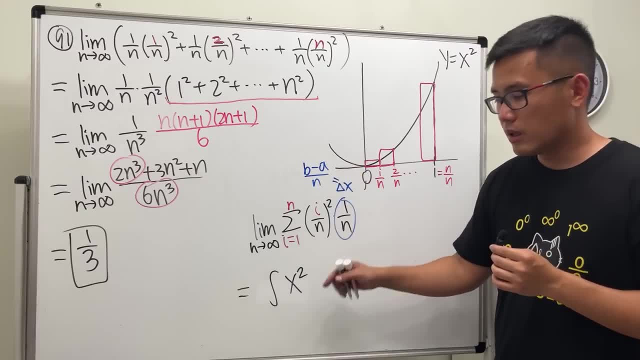 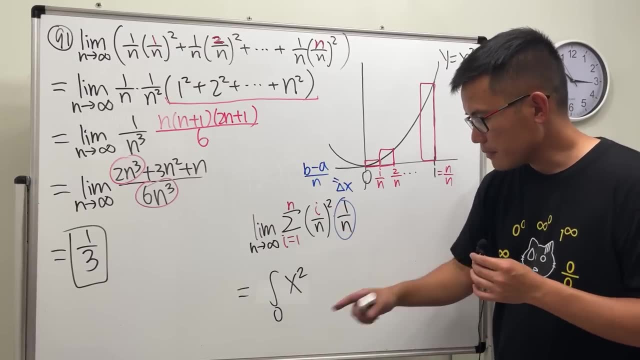 based on this, we know b minus a is 1.. so just go ahead and start with 0. you can always start with 0. you will see it in another question later on. so we can just go from 0 to 1 and then the delta x. 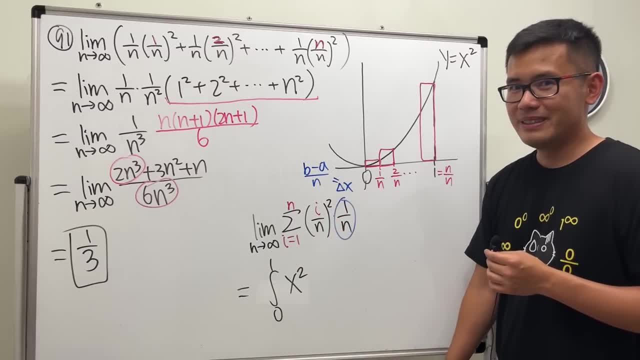 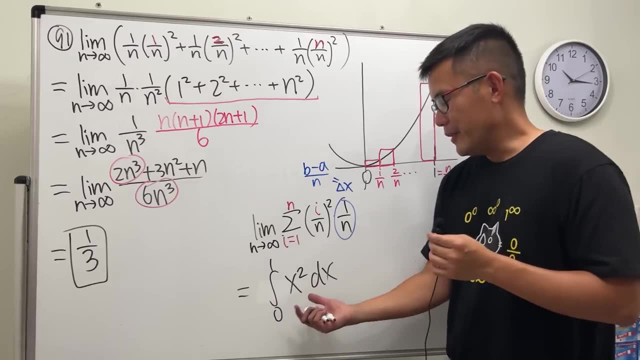 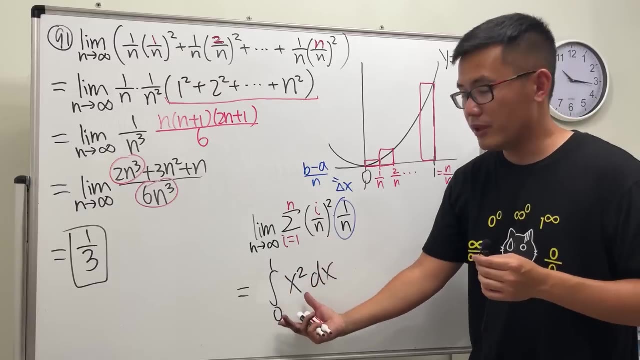 that's so, i don't know. it's 2022 already. don't write delta x, write dx. so anyway, this right here is the explanation of the integral notation. right, so you can ignore that. i want you guys to be able to go from here to here, but of course, it's hard sometimes, so there are a. 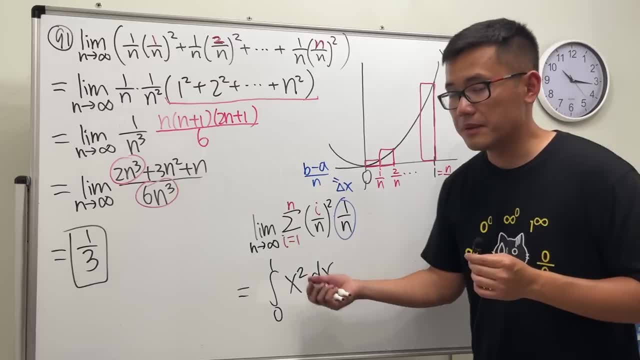 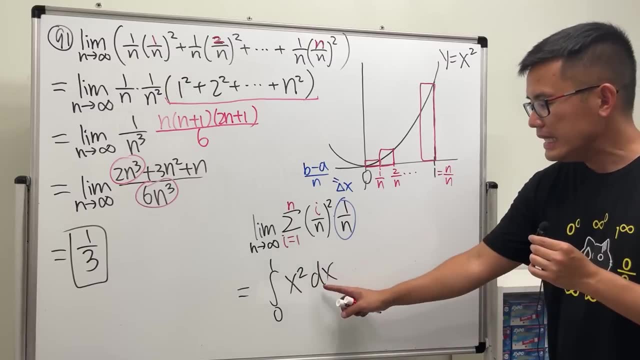 few things that you can do to make sure that you know the integral notation is correct. definitely draw the picture and convince you guys that all the setup is correct. it's correct, though, because you see, we just want the area going from 0 to 1 under x square and the 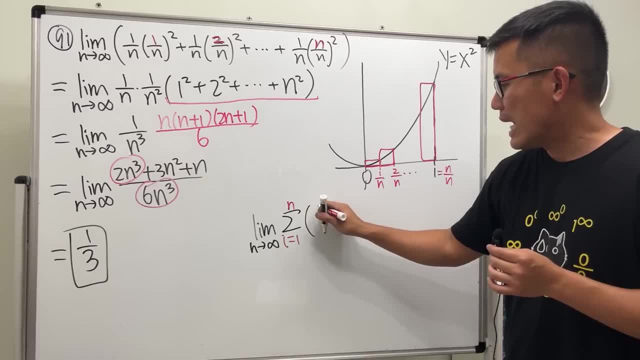 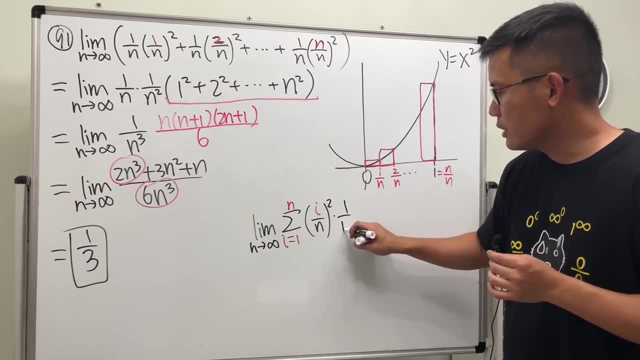 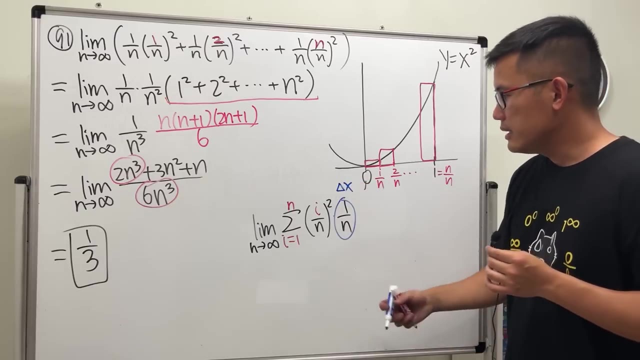 inside. here we have i over n, yeah, and then we square that and then we multiply by one over n. i just put one over at the end. this right here, is the width, aka delta x, delta x. another way to look at it is from where to where, and we write it as b minus. 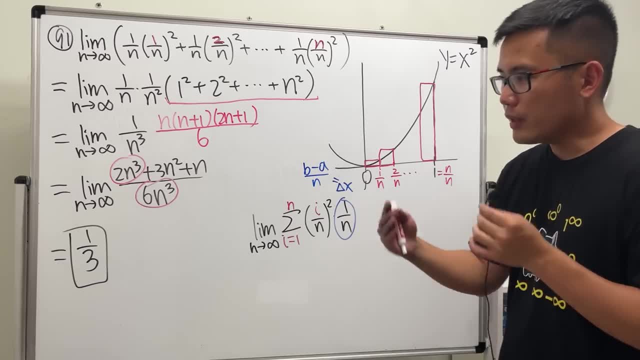 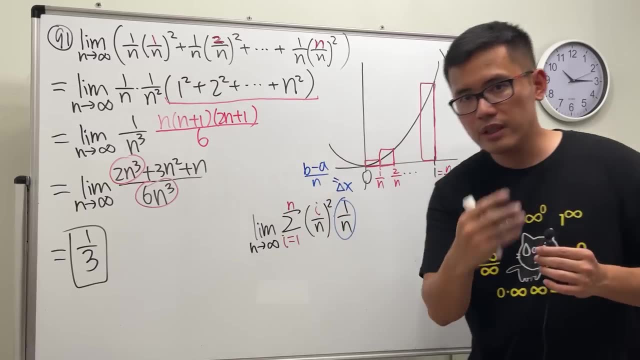 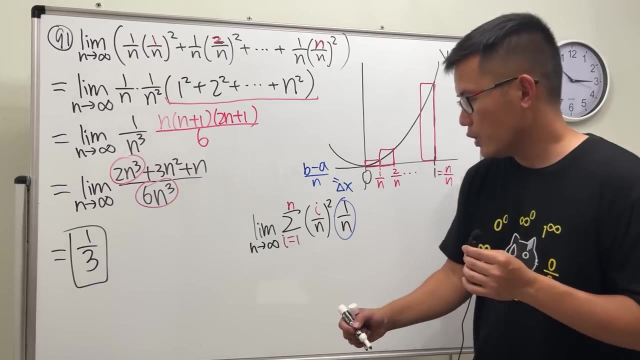 a over n. so the range, right, it's only one unit away. if we start with zero, we end up with one. if we start with seventeen, we end up at eighteen. so that's the structure. and guess what, if you know the structure of this, we can change this to a super version. 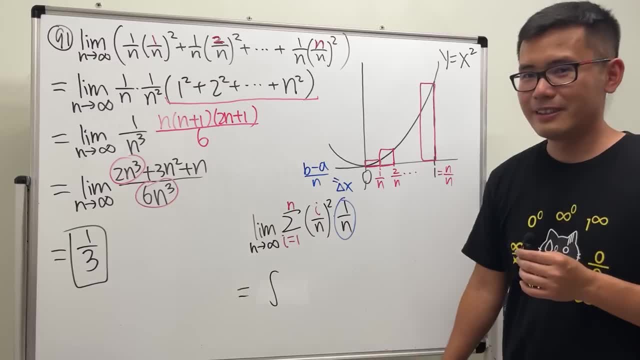 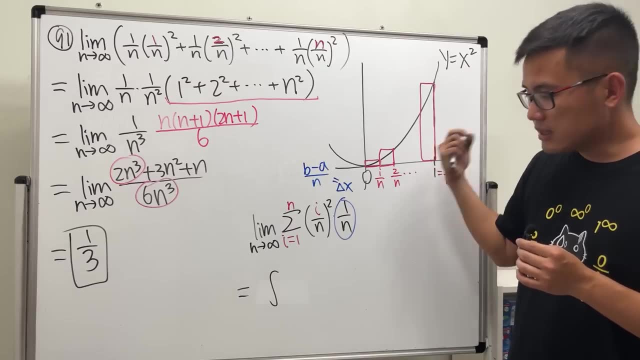 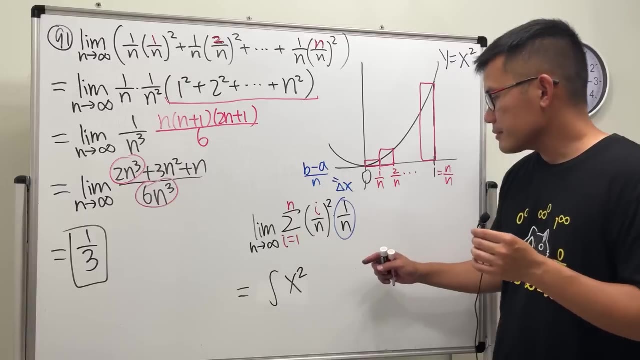 that is the so called integral. what's the function? you see, the input is i over n. that's what we talk about. we enter all this into the x, so that's the function. so the function in this case is x square. yeah, and then you can actually look at it from here. one. 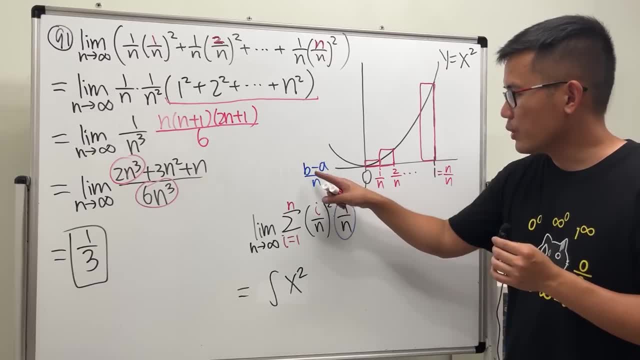 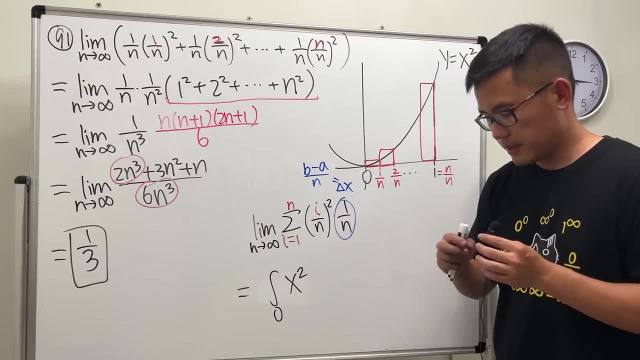 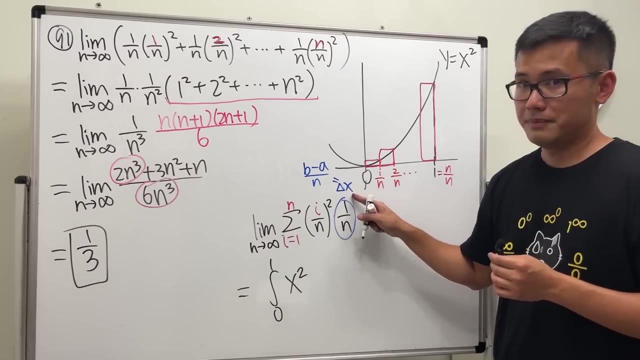 over n. right, and based on this we know b minus a is one. so just go ahead and start with zero. you can always start with zero. you will see it in another question later on. so we can just go from zero to one and then the delta x. 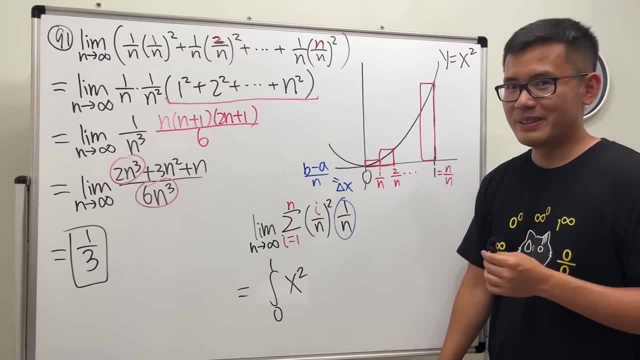 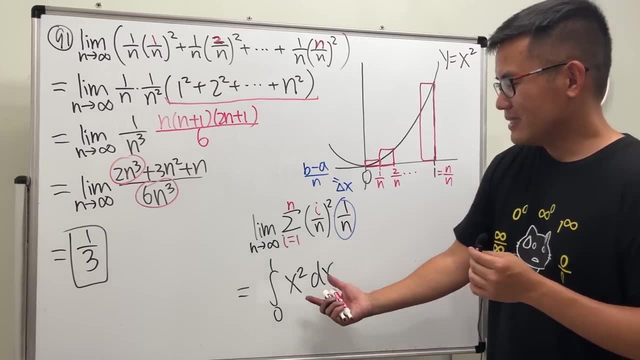 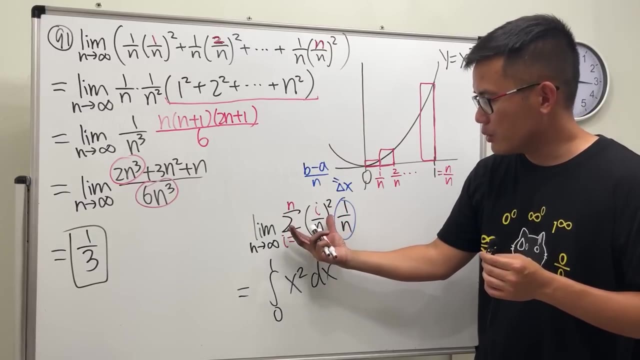 that's so, i don't know. it's 2022 already. don't write delta x, write dx. so anyway, this right here is the explanation of the integral notation, right, so you can ignore that. i want you guys to be able to go from here to here, but of course it's hard sometimes. 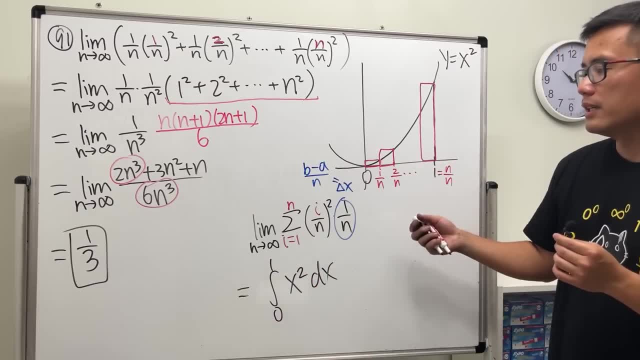 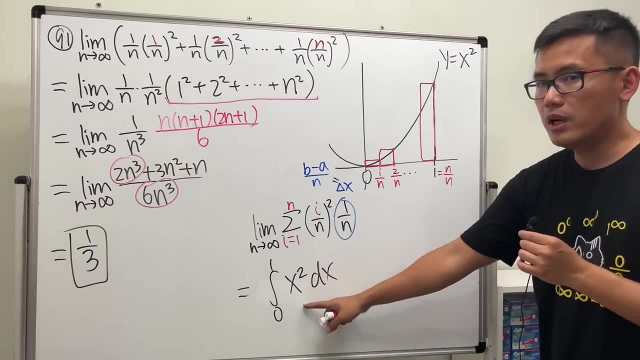 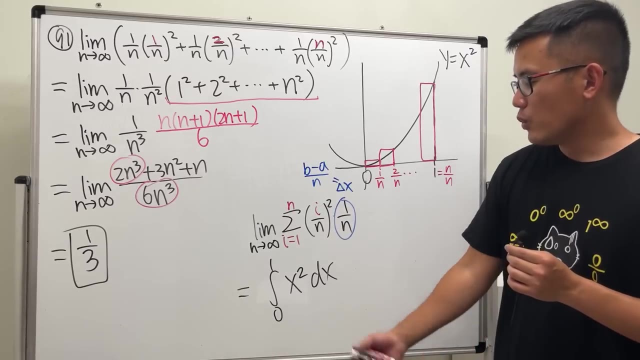 so definitely draw the picture and convince you guys that all the setup is correct. it's correct, though, because, you see, we just want the area going from zero to one under x square, and the dx is just the width of the rectangle. so it does make sense when we have 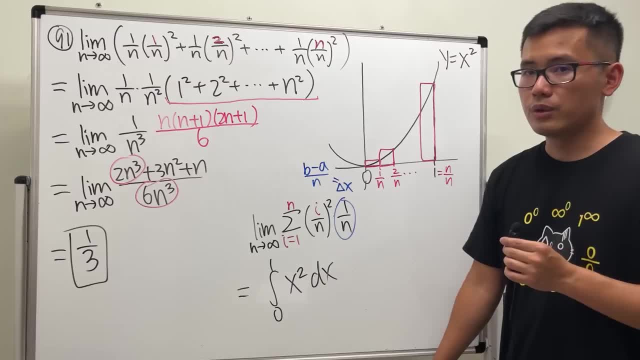 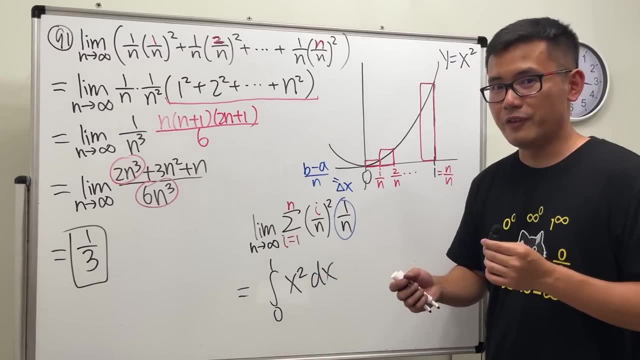 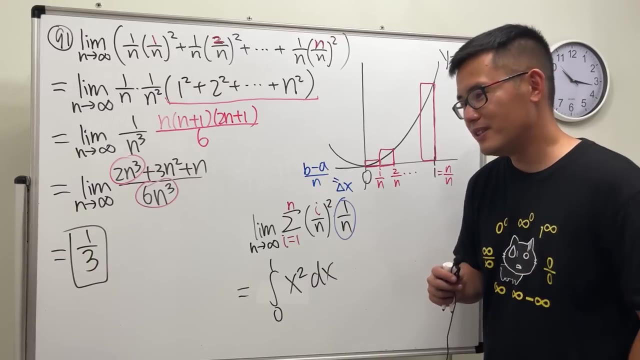 dx is just the width of the rectangle, so it does make sense when we have the dx in the integral notation, right? so how do we do integrals? well, we are going to use the reverse power rule. so if you like this, you can use it for viertex question, or you can use the second one which i will show you. 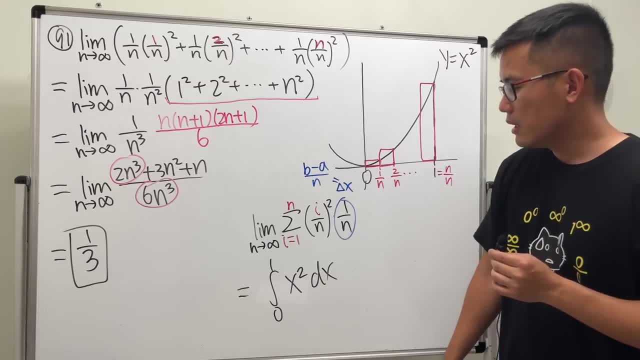 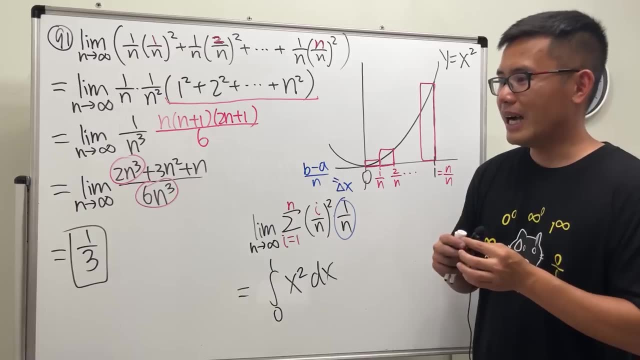 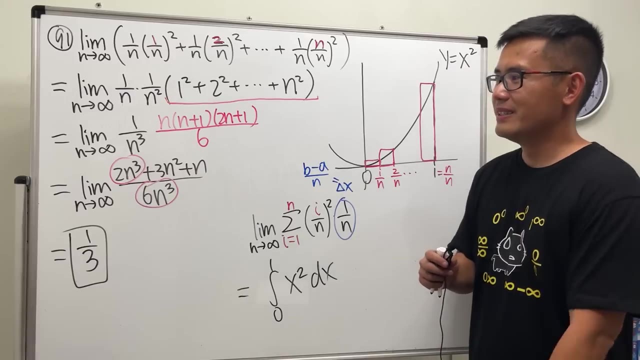 the dx in the integral notation, right? so how do we do integrals? well, we are going to use the reverse power rule. so if you haven't learned about the integrals by now, you can watch my 100 integrals video or you can pause for a little bit. for now, 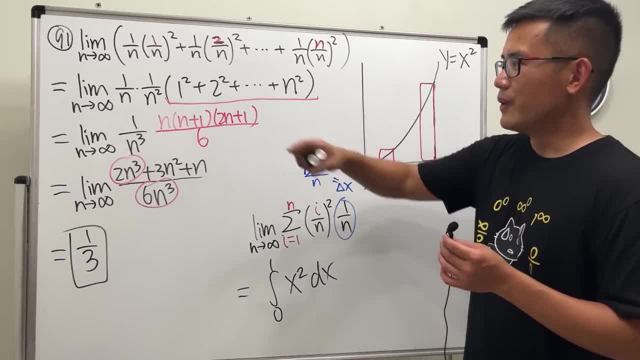 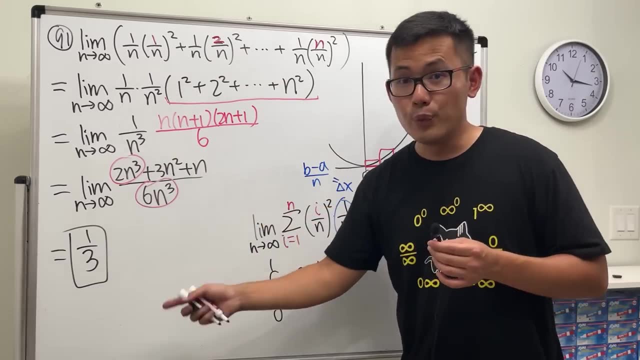 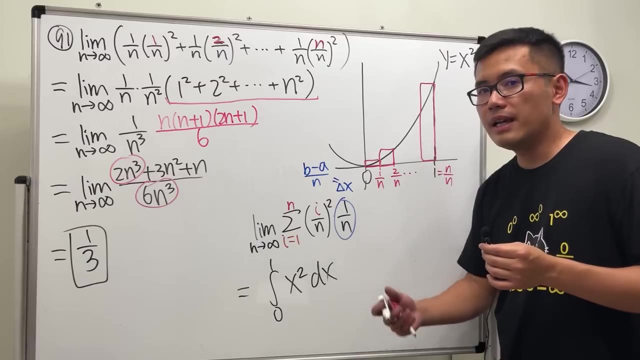 at the end of this video, but for now you can watch my 100 integrals video or you can pause for a little bit. for now, if you are in calc 1, then this is what you have to focus on, and maybe come back after a week or two. then this is what you will be doing. anyway, we use the reverse power rule, meaning 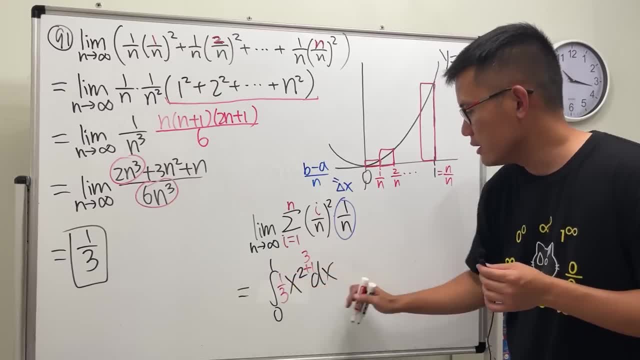 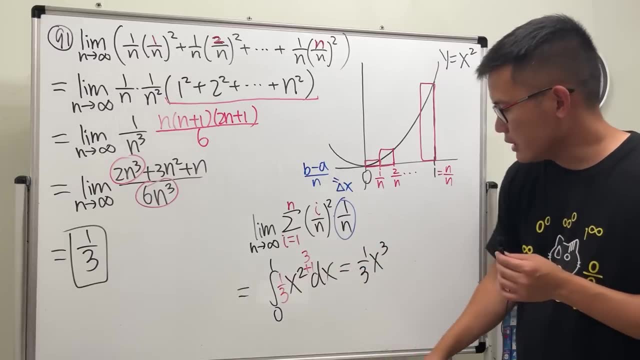 that we find the entire derivative, add 1 to the power, which is 3, and then divided by the new power, for that is just one over three, x to the third power, and then we're going to plug in, plug in, plug in one, and then subtract, plug in zero. this process is called the fundamental. 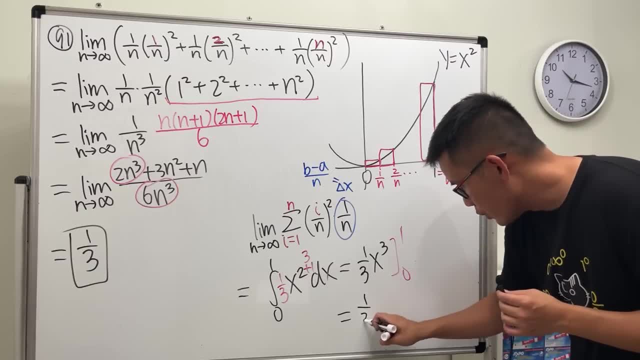 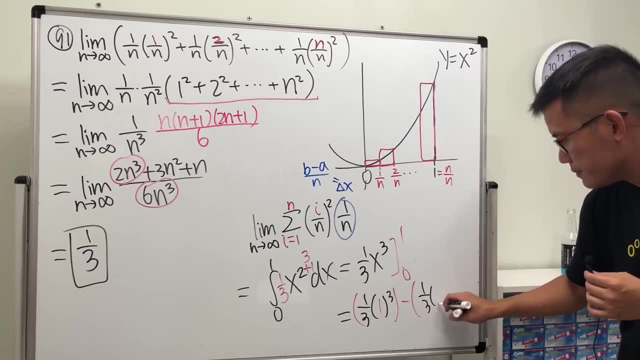 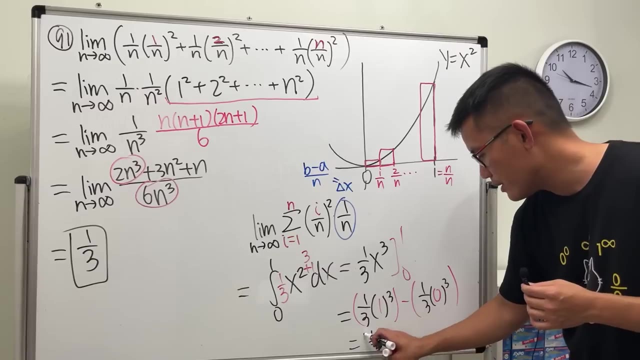 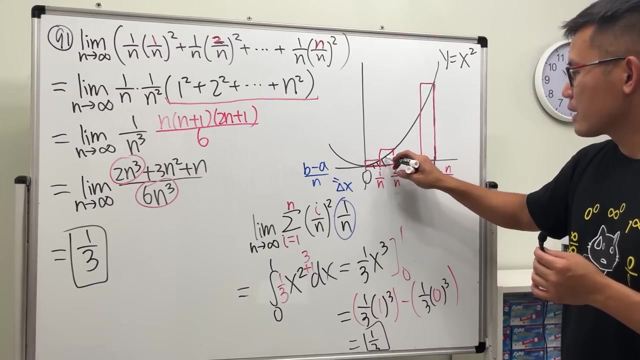 strong calculus, part two. anyway, i'll show you one over three. one to the third power. this is the first part. minus plug in zero, we have one over three, zero. third power: this is zero. this is, yes, you know it, one third. so yeah, this weird curve shape has the area of a very nice number. one third. 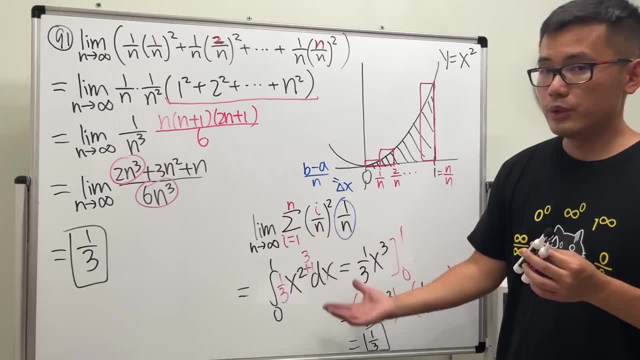 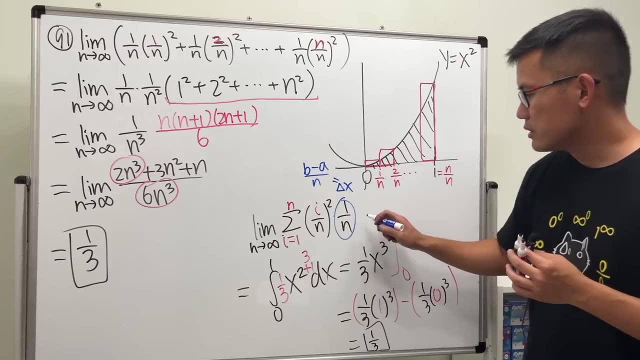 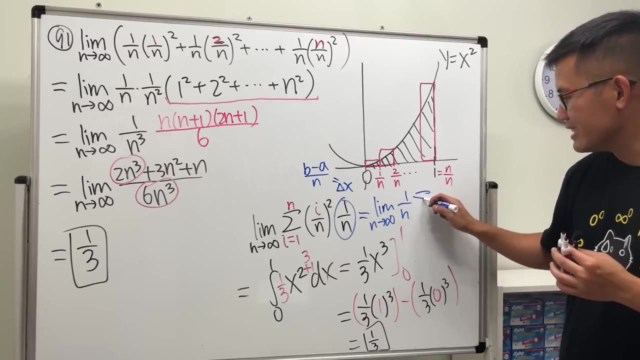 right. so keep in mind of how we go from here to here. but i want to point you guys, though a lot of times the questions will put one over to here, so you will see, we have the limit death, and goes to infinity andِّ infinity, and then 1 over n, and then the sigma, and then i goes from 1 to infinity and whatever this. 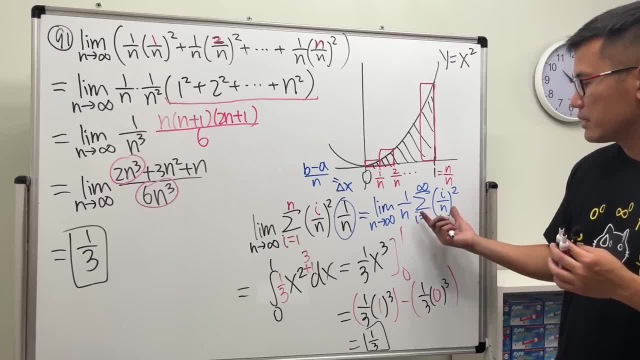 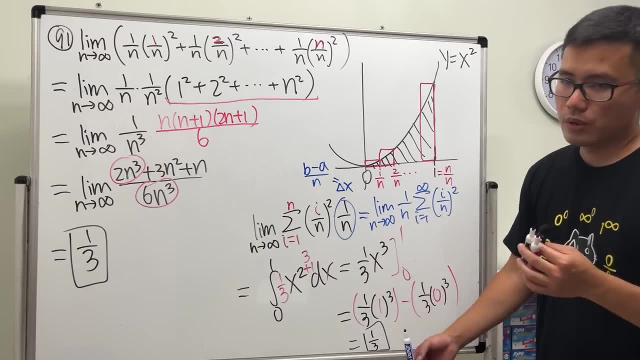 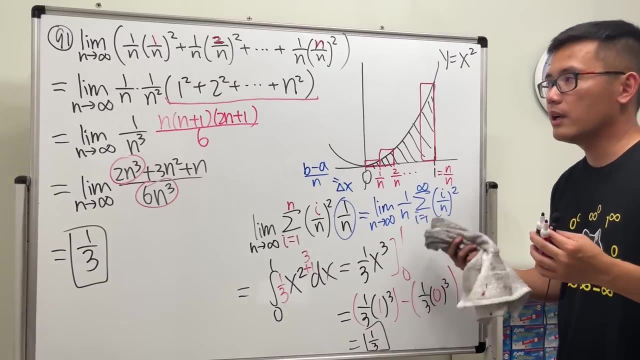 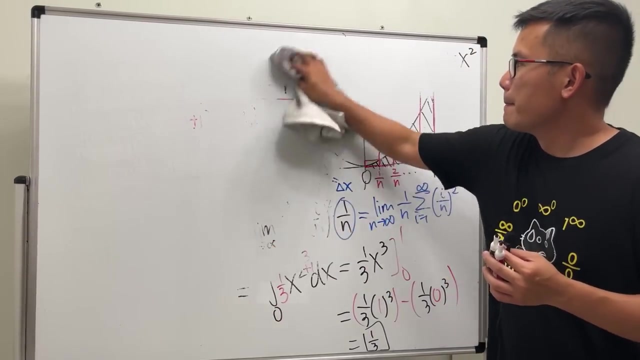 is. but just worry about, this right here will give you the function part. this right here will tell you from where to where and change that to the integral and that's it all right. all right. the next example is going to illustrate why we can always just start with 0. the soda is not. 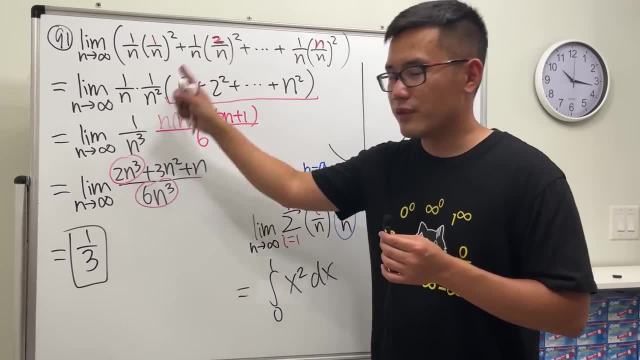 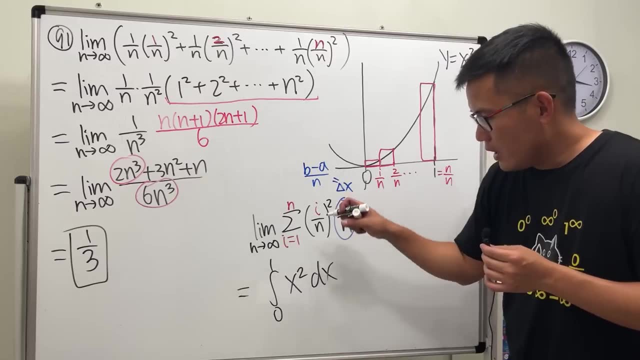 if you are in calc one, then this is what you have to focus on and maybe come back after a week or two. then this is what you will be doing anyway. we use the reverse power rule, meaning that we find the entire derivative. add one to the power. 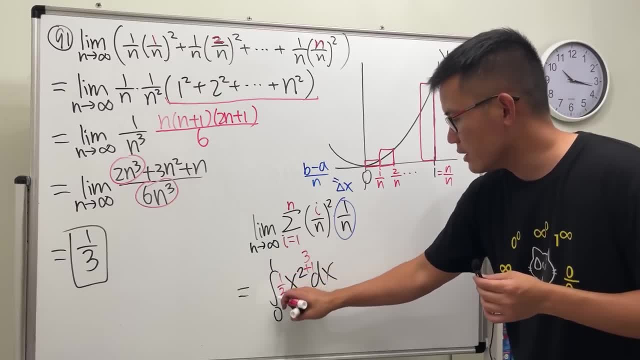 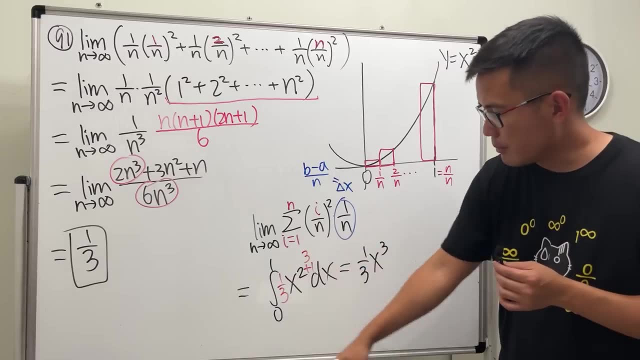 which is three, and then divide it by the new power, so we have one third, so an entire derivative, for that is just one over three, x to the third power, and then we are going to plug in, plug in, plug in one and then subtract, plug in zero this. 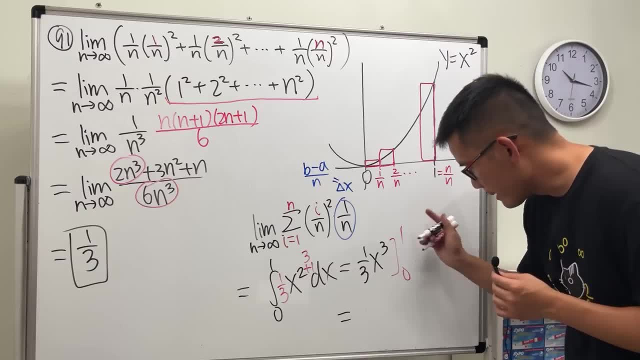 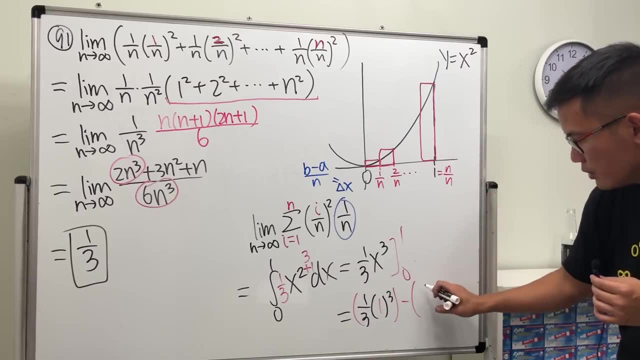 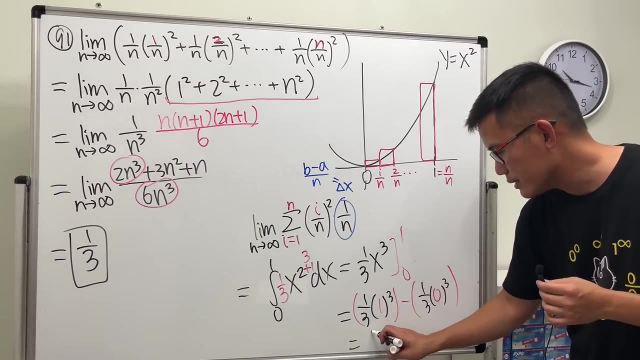 process is called the fundamental theorem of calculus, part two. anyway, i will show you one over three, one to the third power. this is the first part. minus plug in zero, we have one over three, zero. third power, this is zero. this is, yes, you know it, one third. 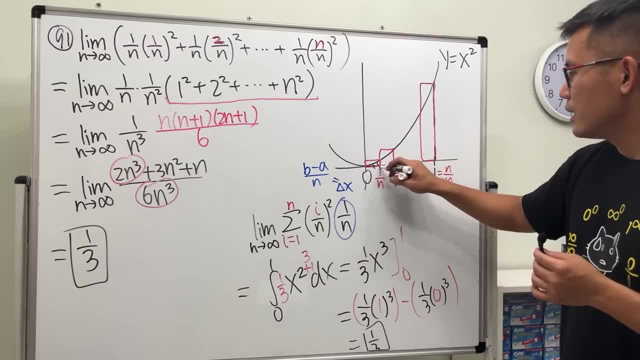 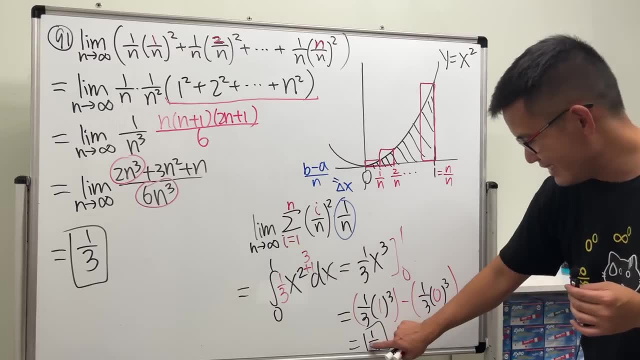 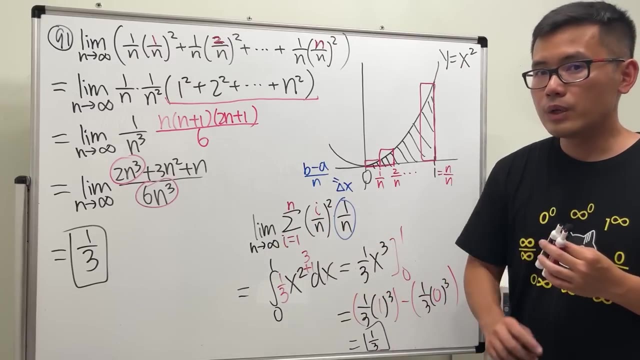 so, yeah, this weird curve shape has the area of a very nice number one. third, all right. so keep in mind of how we go from here to here. but i want to warn you guys, though a lot of times the questions will put one over to here. so 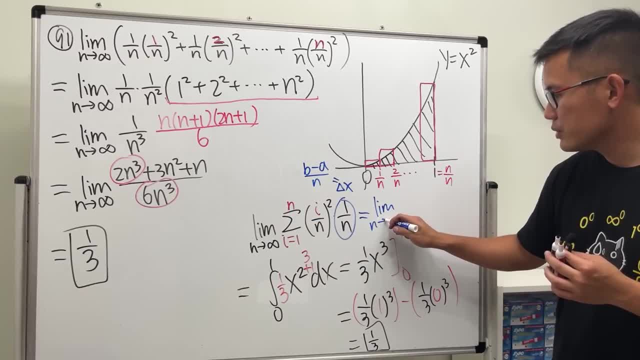 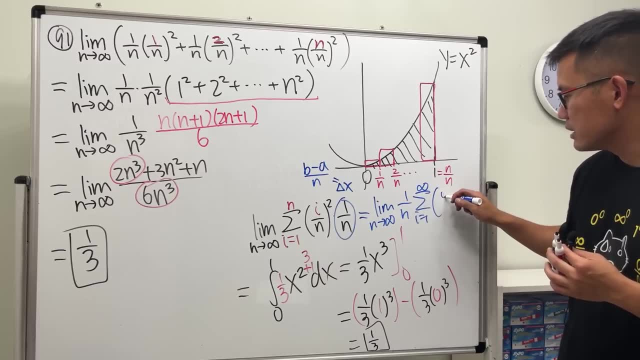 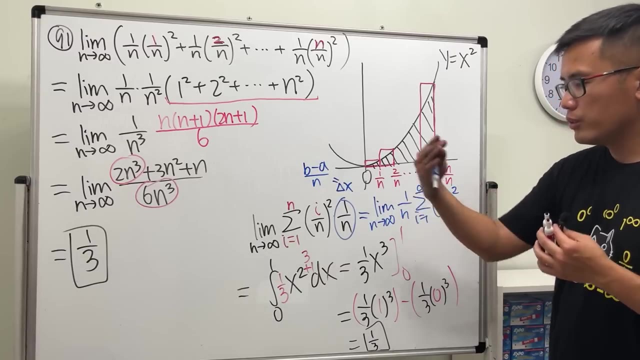 you will see, we have the limit, as n goes to infinity, and then one over n, and then the sigma, and then i goes from one to infinity, and then whatever this is. but just worry about, this, right here will give you the function part. this way he will tell you from where. 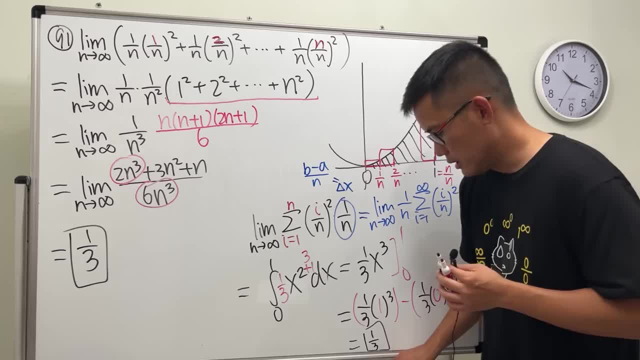 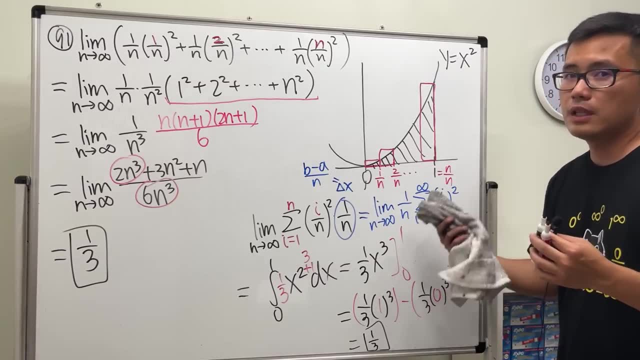 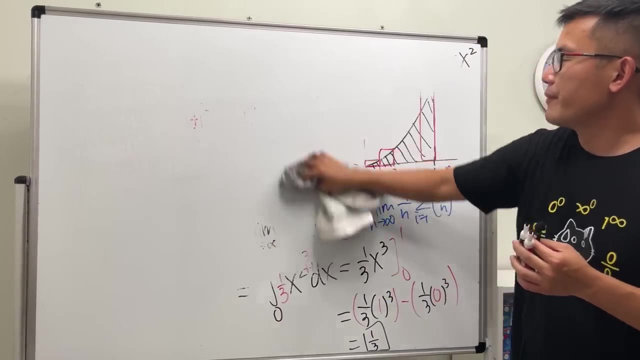 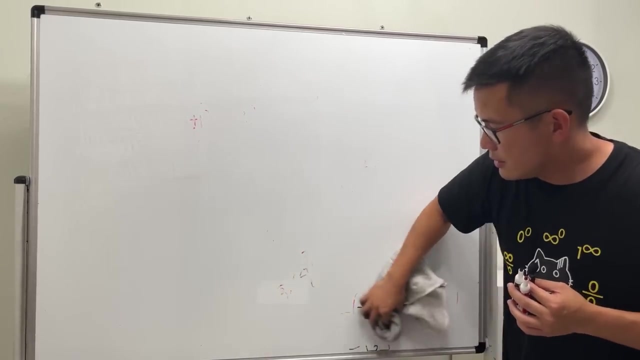 to where and change that to the integral and that's it all right, all right. the next example is going to illustrate why we can always just start with zero. the soda is not cold anymore, so i'm i don't know if i should finish it. anybody wants it? 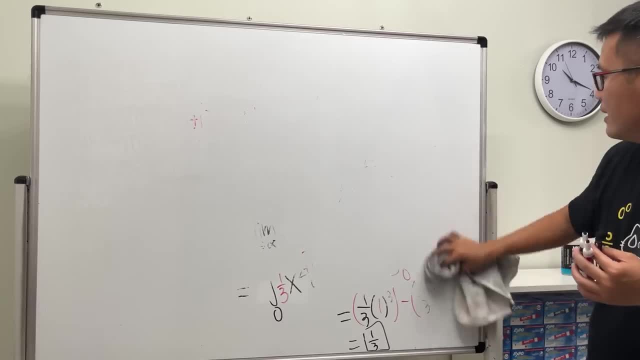 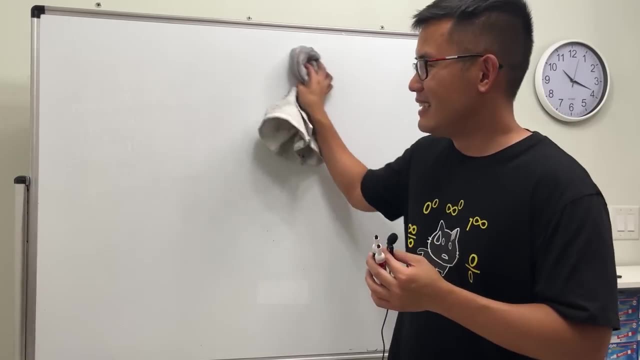 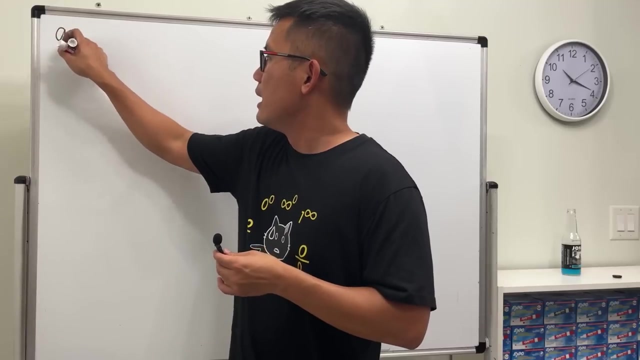 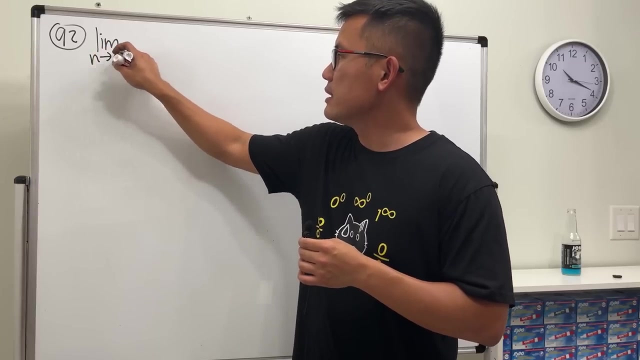 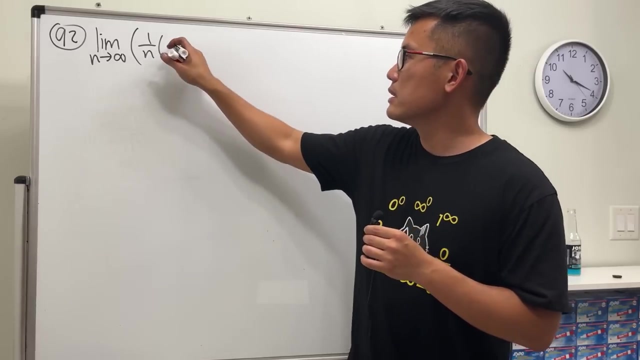 cold anymore, so I'm I don't know if I shall finish it. anybody wants it. probably not, don't, okay? and number 92. yeah, it's very similar to earlier. you will see. this is the limit, as X up, X n goes to infinity, and then we have 1 over n, and then we are going to have 2 plus 1 over n. 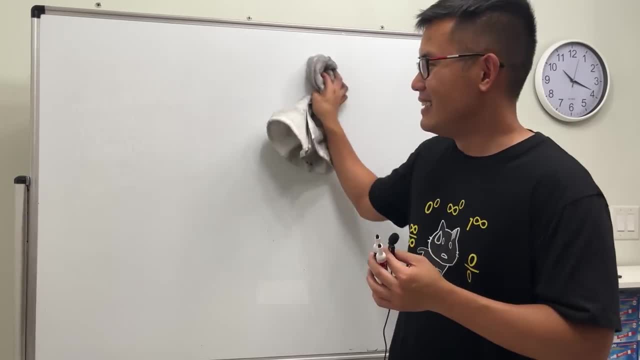 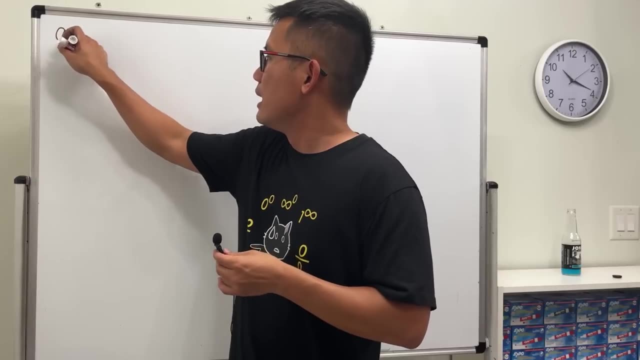 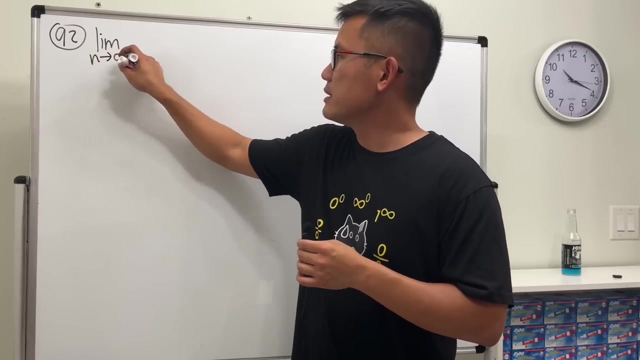 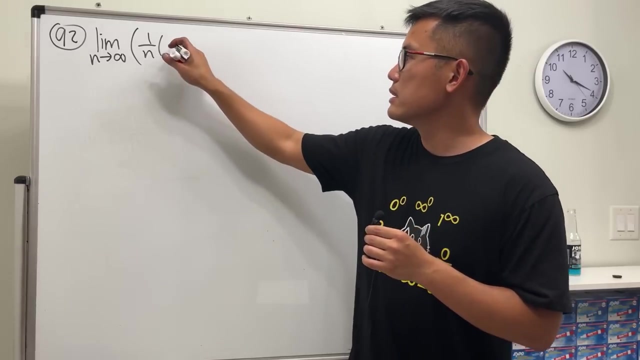 probably not. don't okay, number 92. here it's very similar to earlier. you will see, this is the limit as x of xn goes to infinity, and then we have one over n, and then we are going to have two plus one over n, squared, and the next one over n. 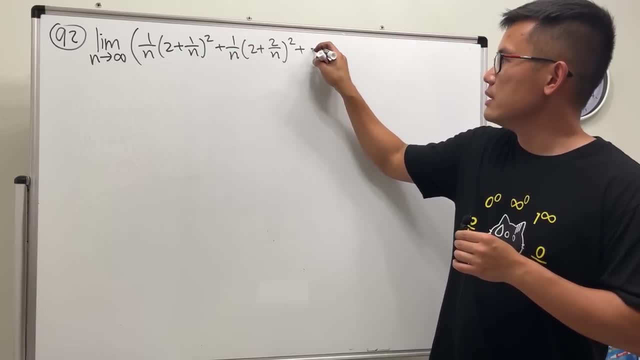 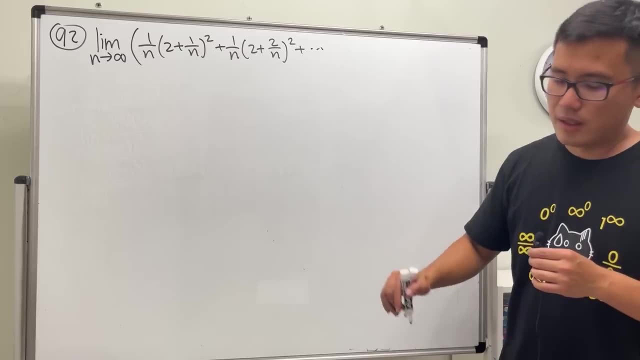 times two plus two over n, squared, and so on, so on, so on- the next one will be here: two plus two over n and all that stuff. okay, you can see on the handout, but i'm just not writing it down. and then one over n, two plus. 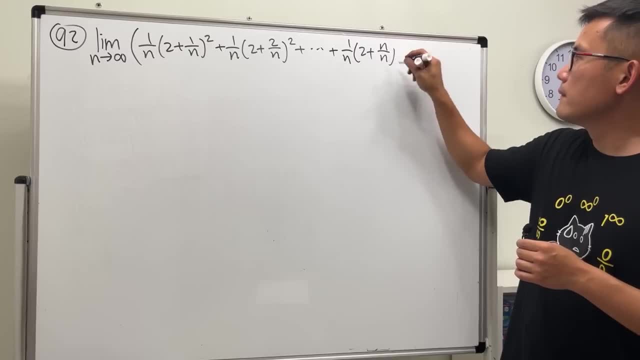 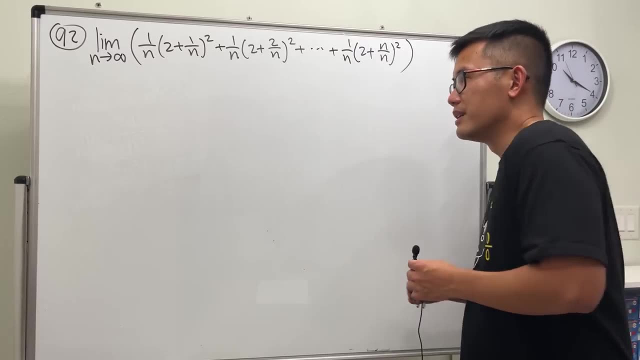 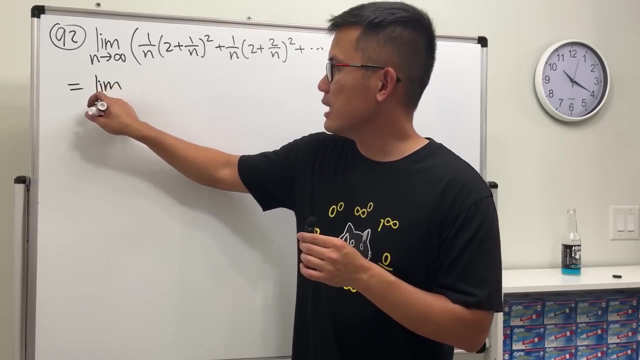 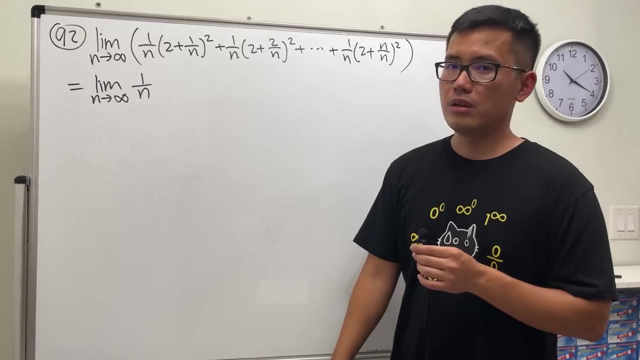 n over n, squared, all right. so here we go. let's combine this into a sigma notation. it will be the limit, as n goes to infinity. everybody has one over n. we can factor it and then, you see, i'm going to put it right here, okay, usually. 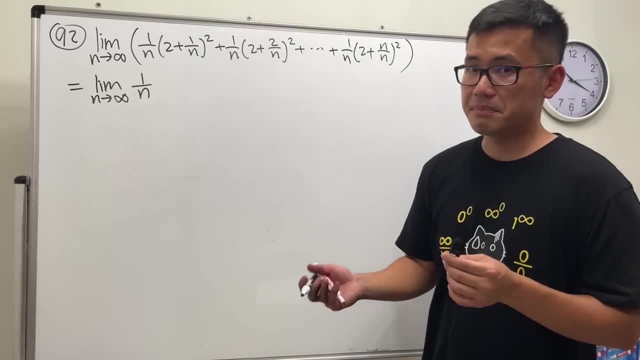 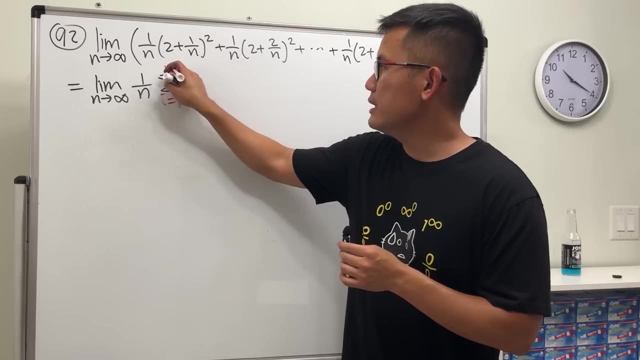 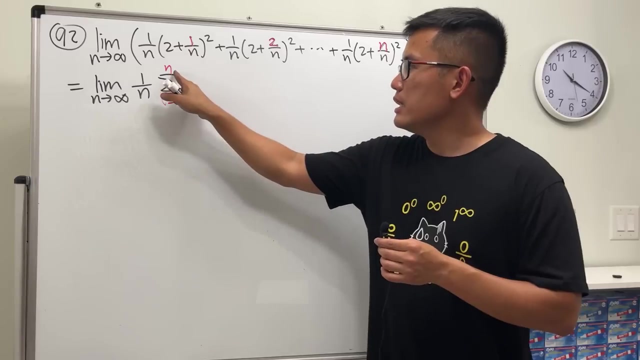 nobody really put it at the end, but that's the dx part. you just have to realize that, and then we have the sum. i goes from one to n and i is this: one, two, three, four and so on up to n. that's the changing part, and this time 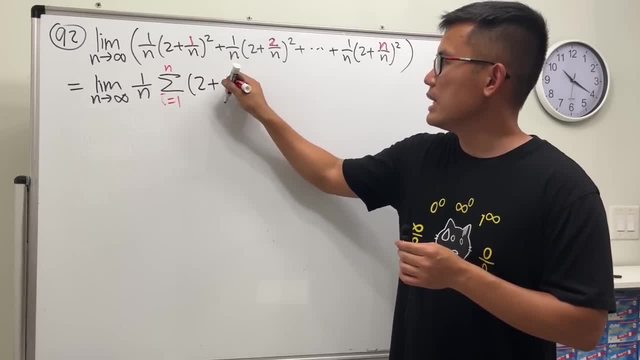 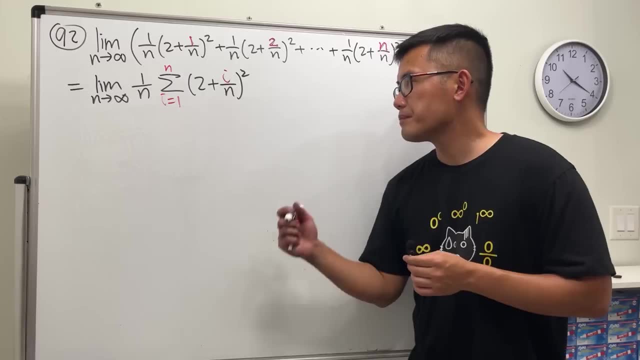 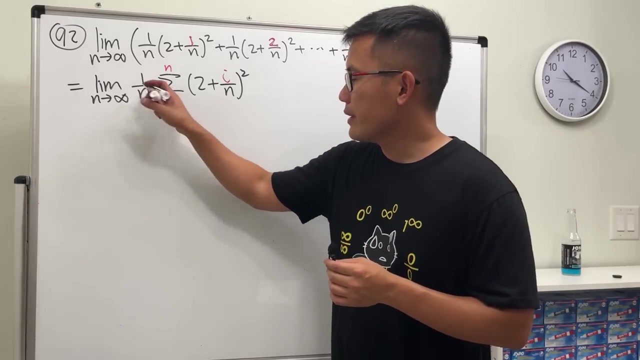 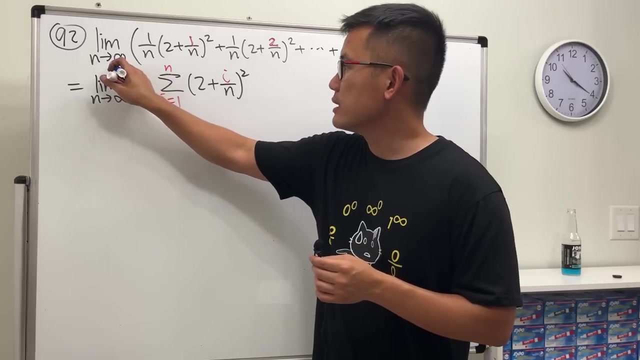 you see, we have two plus i over n, and then squared. okay, now, based on this, what region are we talking about? well, again, let's focus on this right here. first, we have one over n. huh, so this right here tells us: b minus a will give us one. 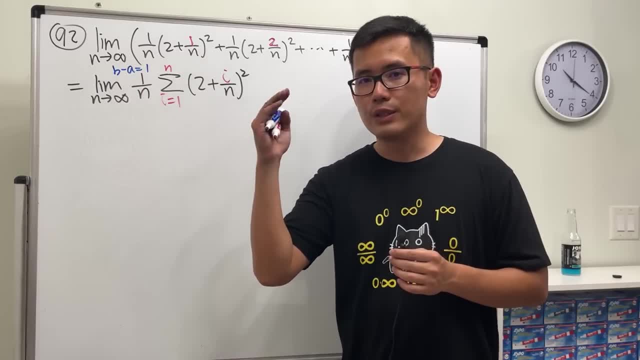 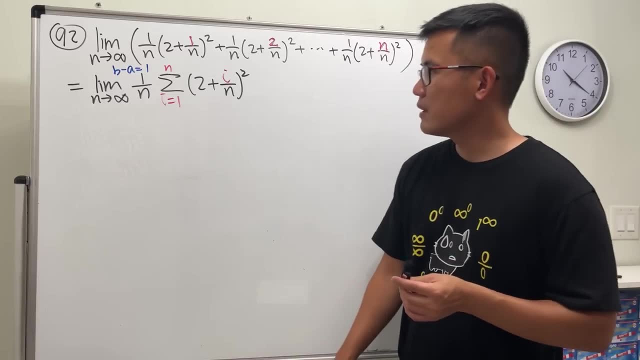 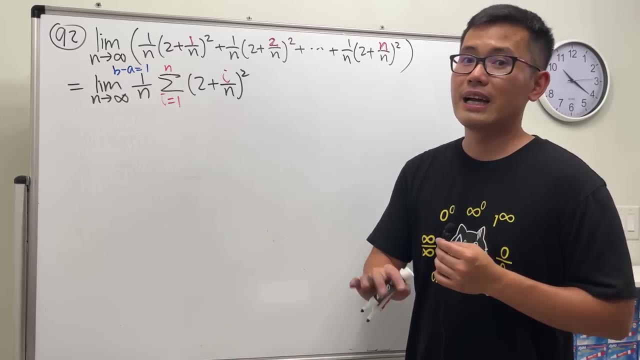 if we start with zero, we end with one. if we start with twenty five, we end up with twenty six, et cetera, et cetera. all right, does that help? not really. okay, just start with zero, that helps. just start with zero, that helps, okay, just. 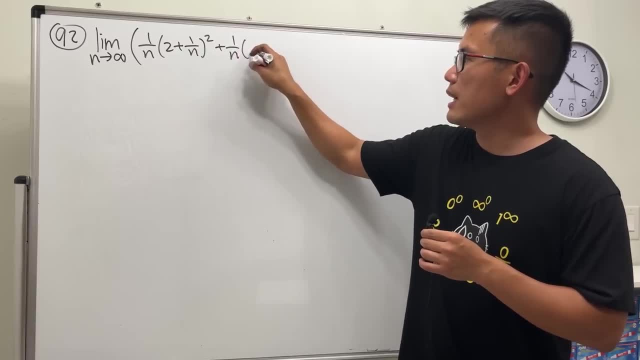 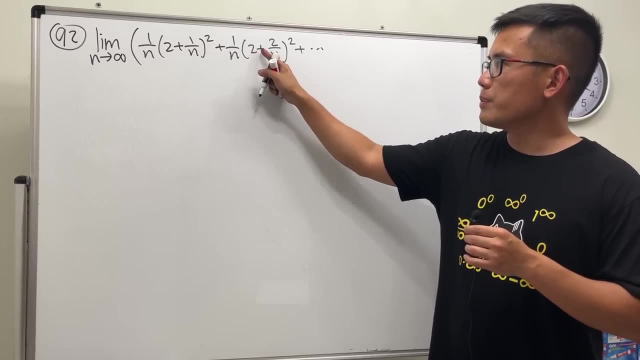 squared, and the next 1 over n times 2 plus 2 over n, squared, and so on, so on, so on. the next one will be here, 2 plus 3 over n, and then all that stuff. okay, you can see, I am handle, Sam, just not right now. this is $ отдue for your question, something here. in this case it's F if the S, i'm alguna. 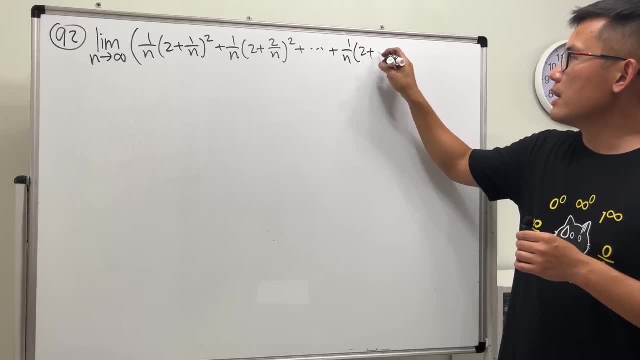 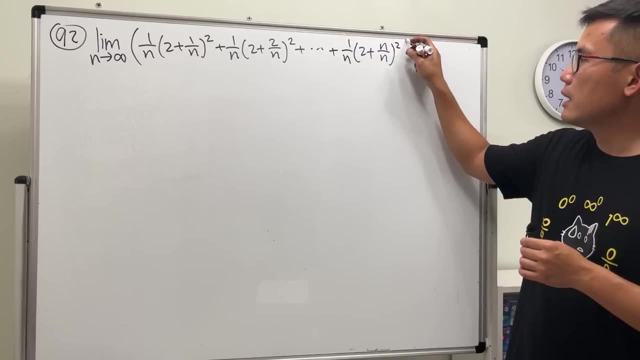 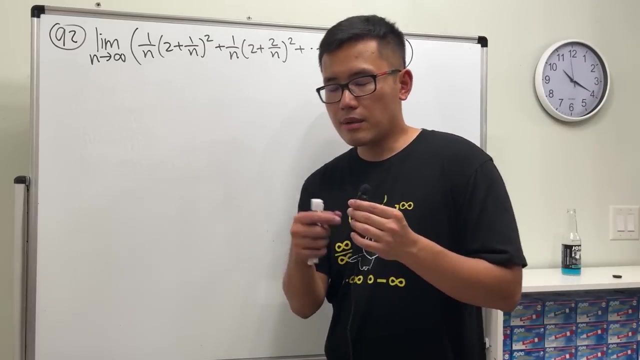 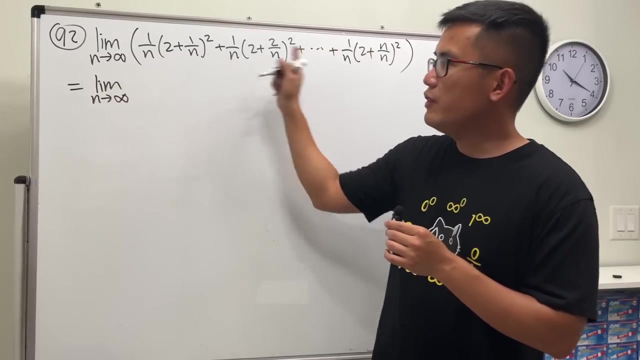 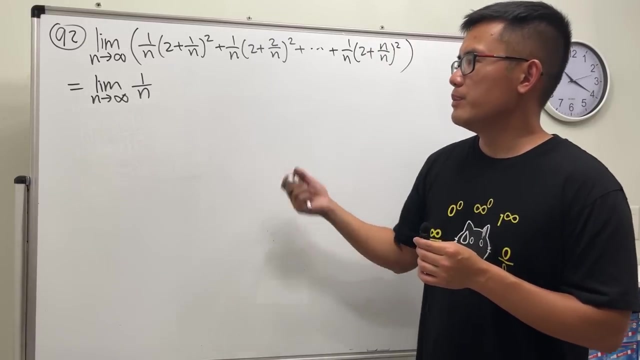 it down and then 1 over n, 2 plus n over n- square. all right, so here we go. let's combine this into a sigma notation. it will be the limit, as n goes to infinity. everybody has 1 over n. we can factor it and then, you see, i'm going to put it right here. okay, usually nobody really put it at the end. 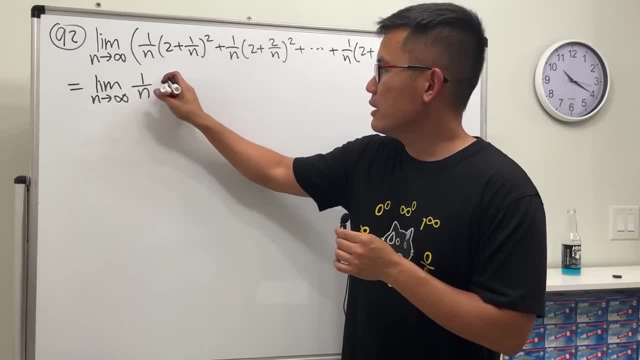 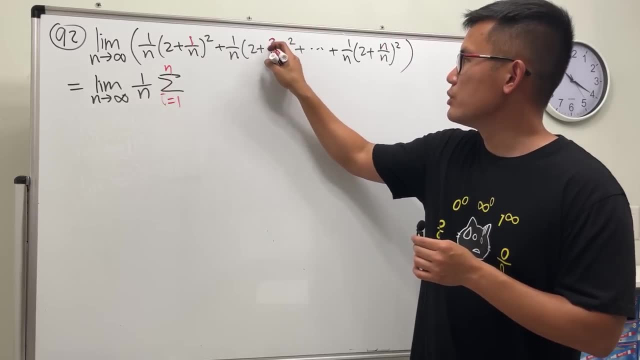 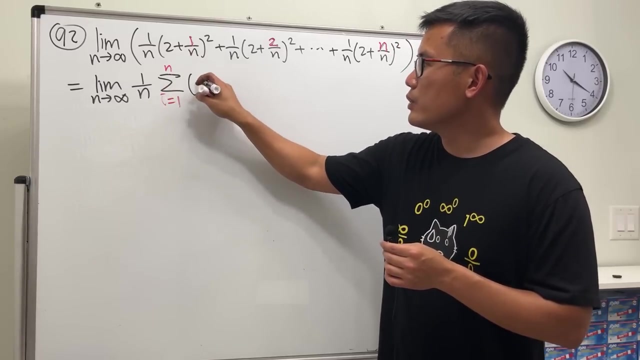 but that's the dx part. you just have to realize that. and then we have the sum. i goes from 1 to n, and i is this: 1, 2, 3, 4 and so on up to n. that's the changing part, and this time you see we have 2 plus i over n and then square. 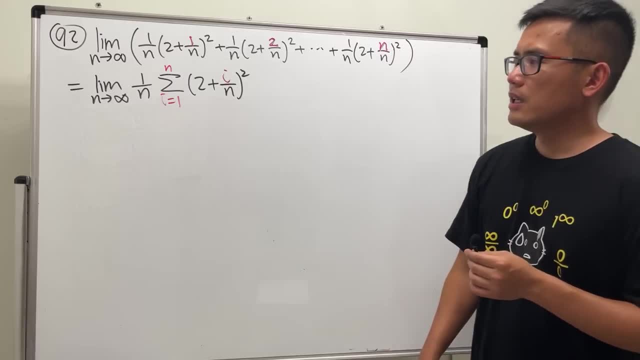 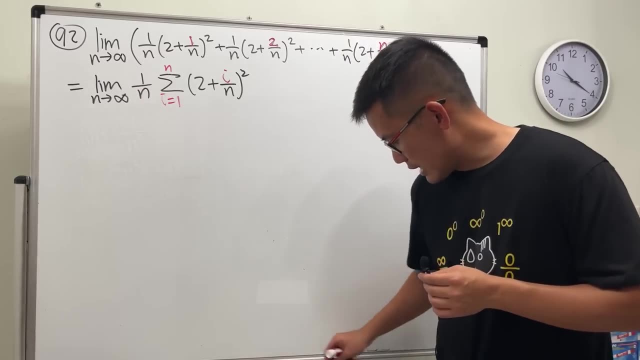 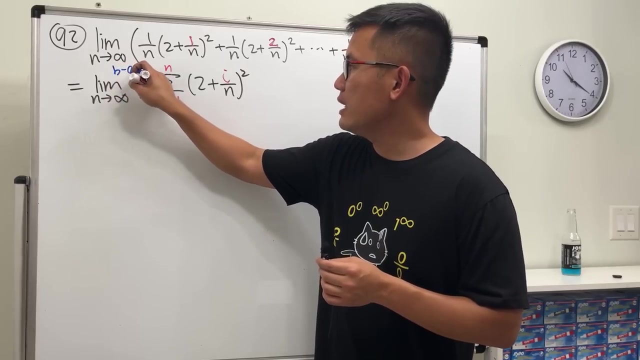 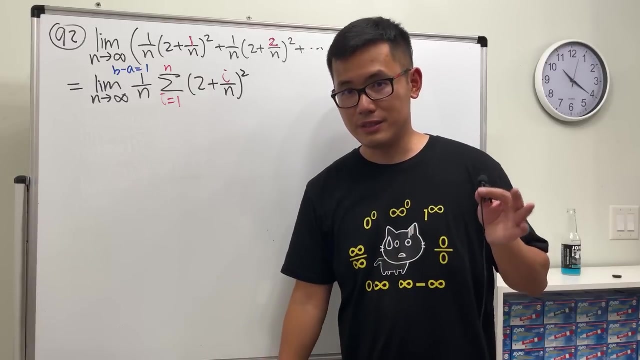 okay, now, based on this, what region are we talking about? well, again, let's focus on this right here. first, we have 1 over n. huh, so this right here tells us: b minus a will give us 1.. if we start with 0, we end with 1. if we start with 25, we end up with 26. 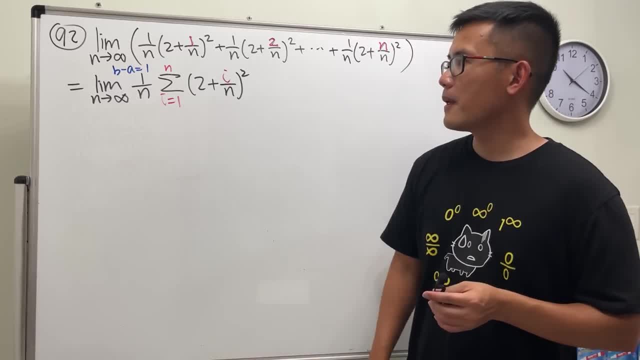 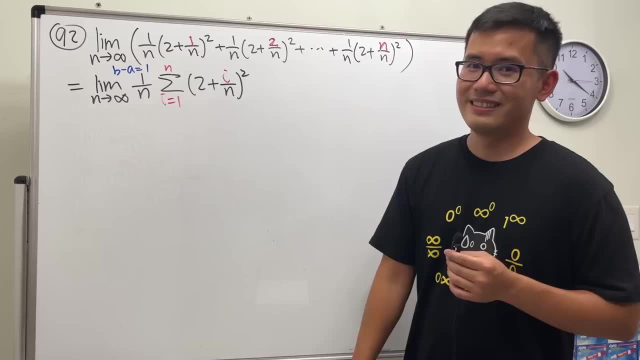 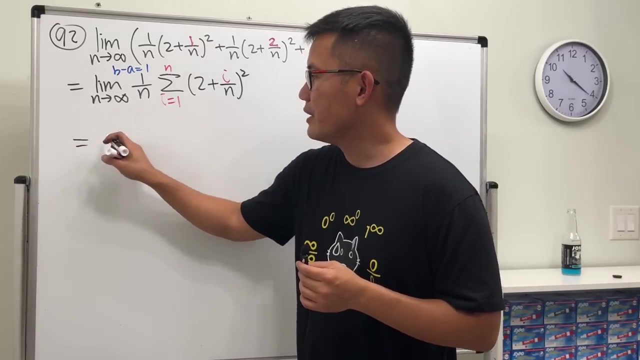 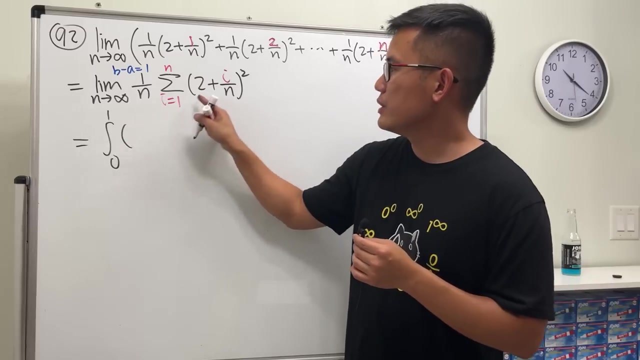 etc, etc. all right, does that help? not really. okay, just start with 0. that helps. just start with 0, that helps. okay, just start with 0.. so i'm going to claim that this, right here, it's actually just the integral going from 0 to 1. just start with 0.. and then the function is actually 2 plus this, right. 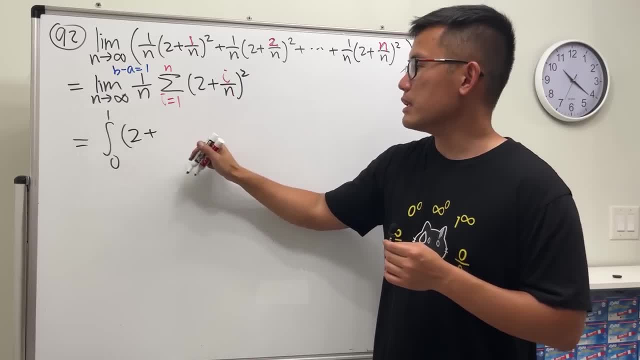 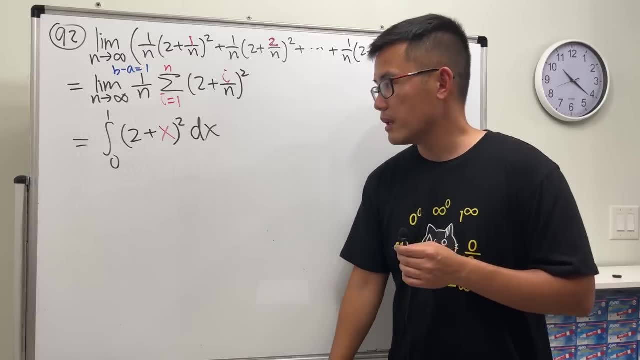 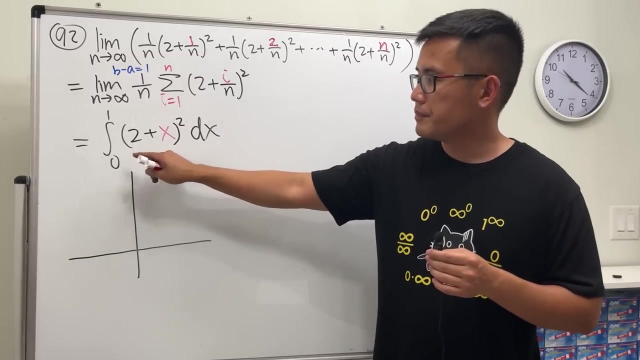 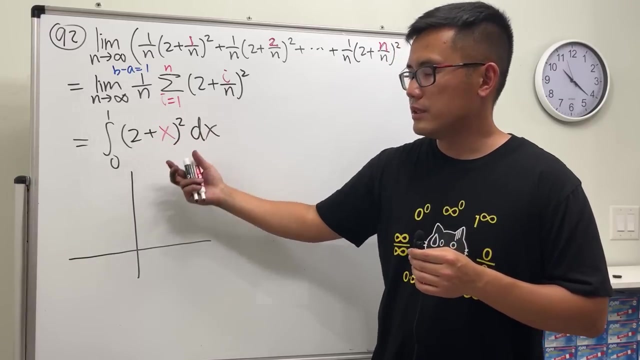 here i over n, it's just going to be the x and then square and then dx, so you can change that to an integral. this integral, of course, represents the following: have a look: if you grab 2 plus x, it's just like so. if you grab 2 plus x squared, it's just like you. 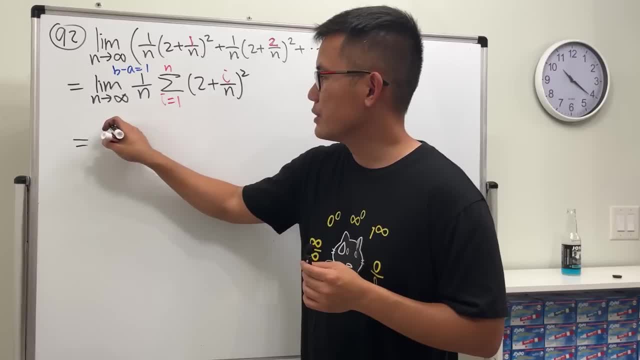 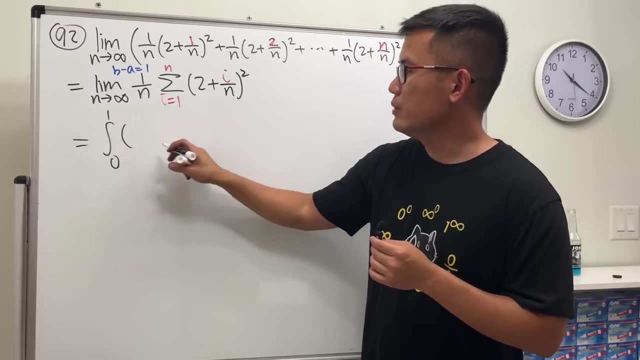 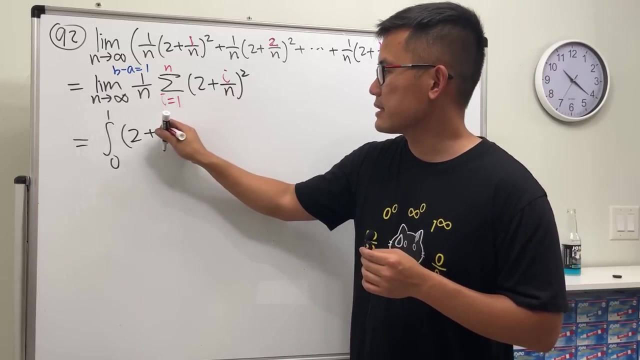 start with zero. so i'm going to claim that this, right here, it's actually just the integral going from zero to one. just start with zero, and then the function is actually two plus this, right here, i over n, it's just going to be the x and then square. 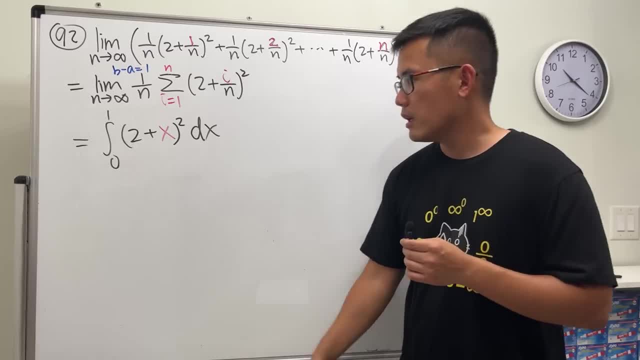 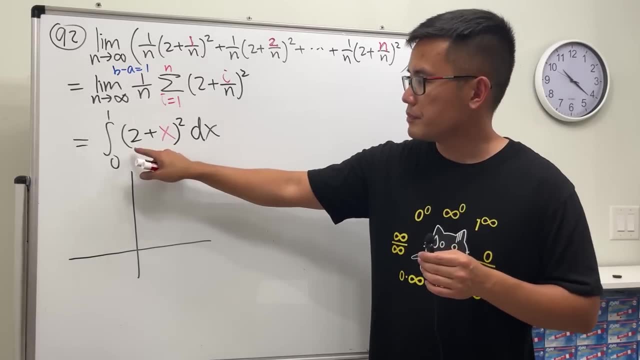 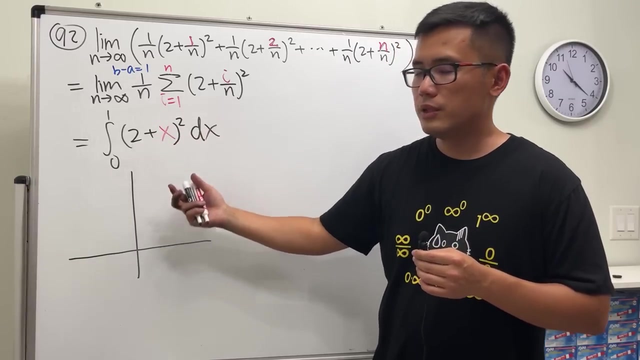 and then the x, so you can change that to an integral. this integral, of course, represents the following: have a look, if you grab two plus x, it's just like- sorry. if you grab two plus x squared, it's just like you have a parabola but you put to the left. 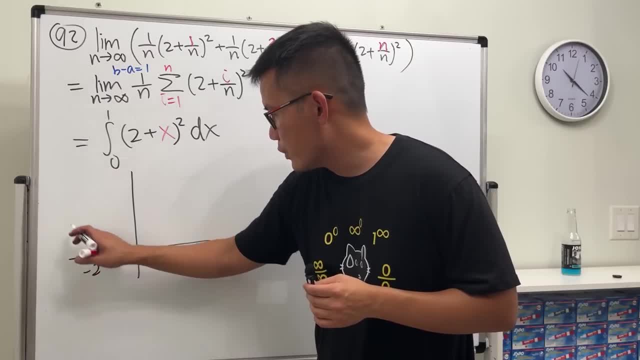 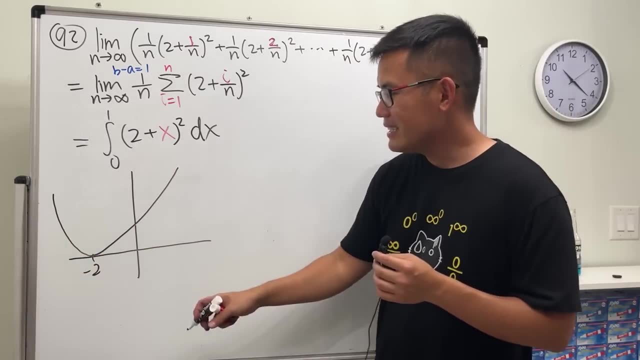 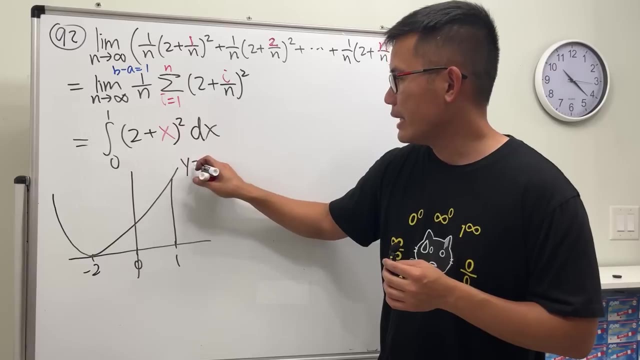 two units, right, so when x is negative, two. here we have a parabola, something like this: okay, and i'm saying that the region that we want is from here to here is zero to one. and then have a look, this is: y equals two plus x. 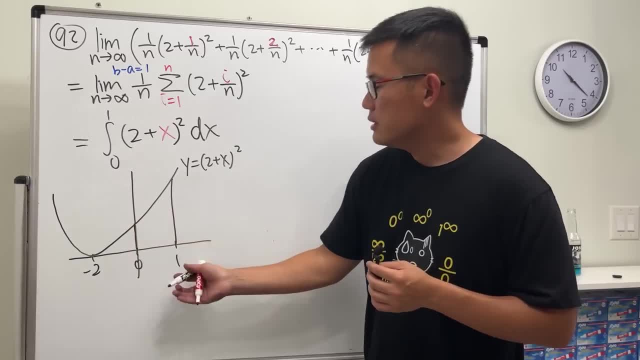 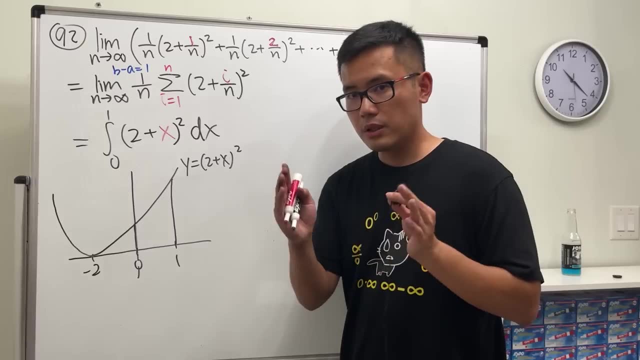 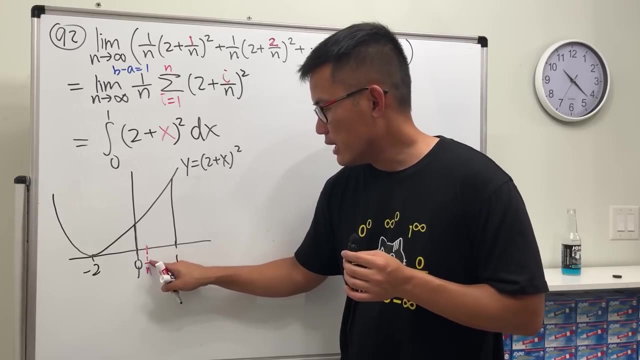 to the second power. does this satisfy our original? it does have. a look. we go from here to here, so the whole thing is one cut into n pieces, so each piece is one over n. so the first x value that we can use is one over n. put it here: 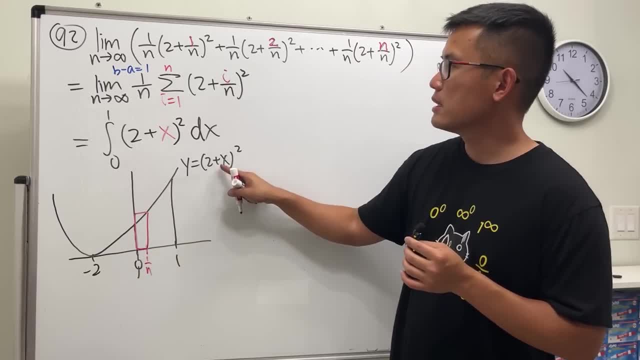 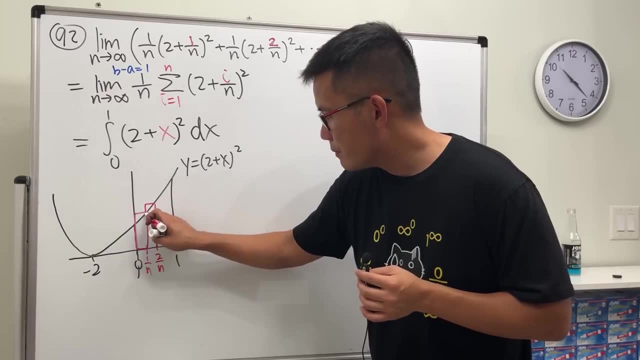 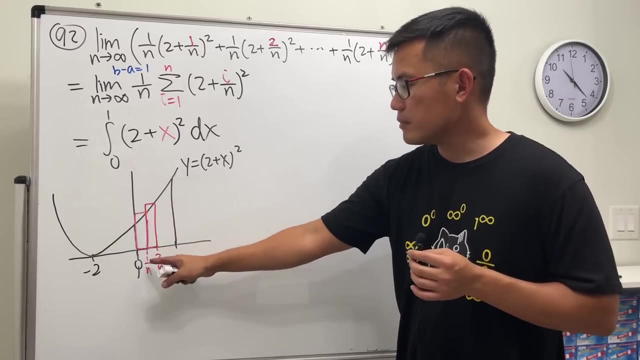 the height is what? one over n in here. so we have two plus one over n squared. the next x value: two over n. put it here: we have two plus two over n squared. that's the height, and then everything here. the width is one over n, so yeah, 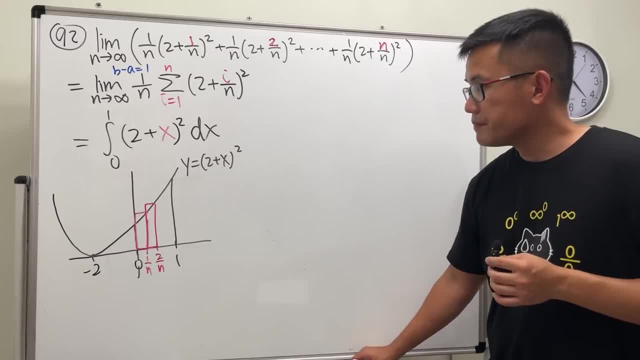 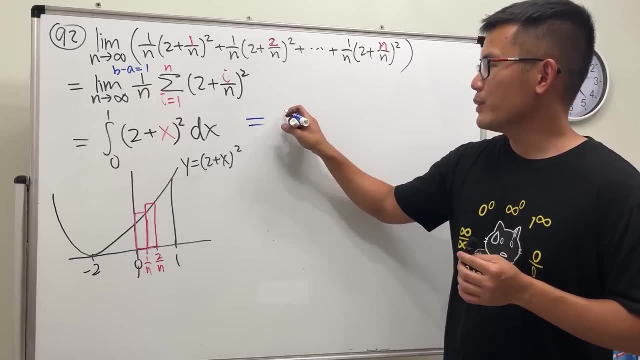 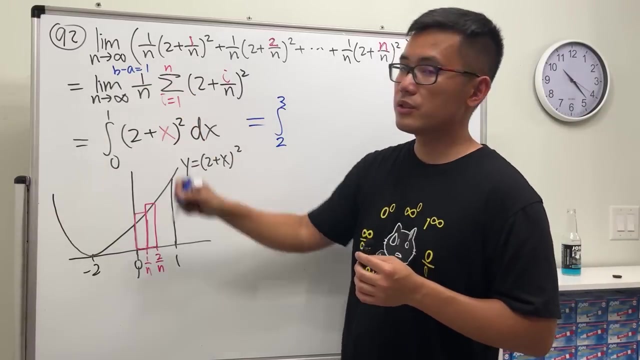 that should convince you guys. huh, okay, what if you don't want to start with zero? i don't know. if you want to start with two, it's okay too, i'll show you. if you start with two, then you go up to three. per our discussion earlier, 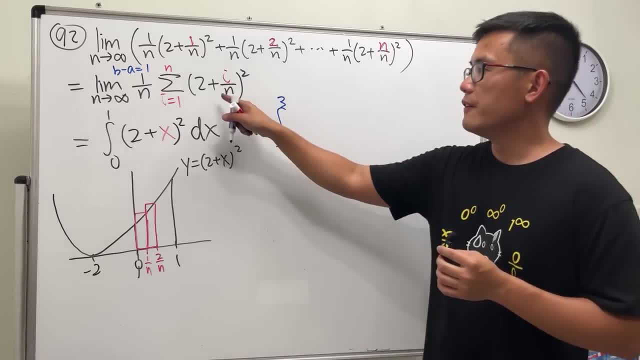 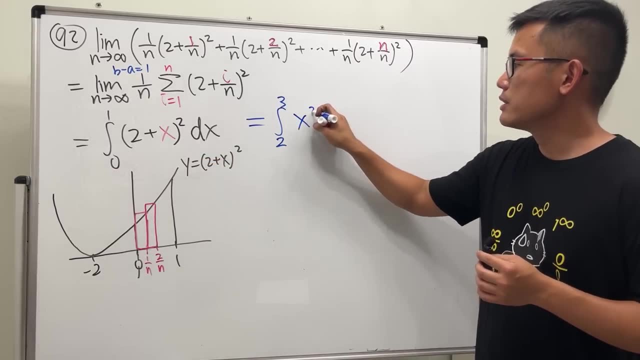 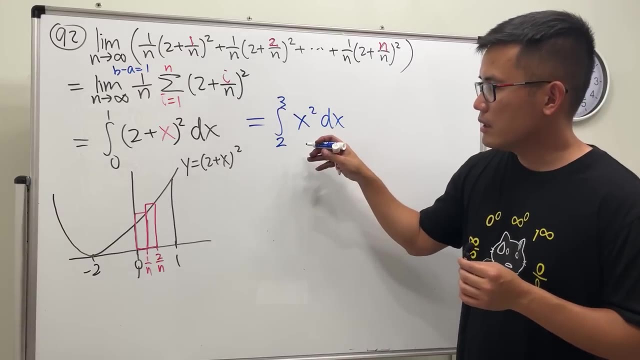 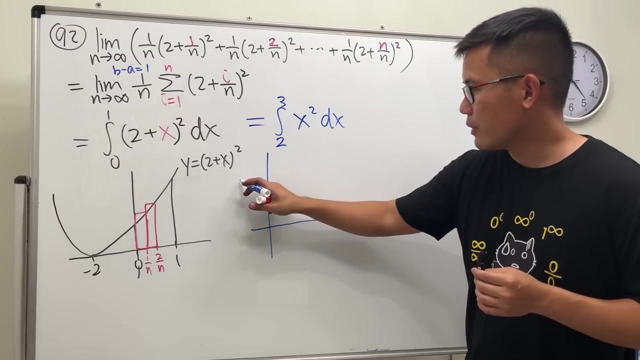 right, and in that case the function is no longer the same. right here. but you put it as just x squared x. why? let me show you this right here. will give you that as well. check this out. so we have our x squared horrible picture. no, i'm sorry, but if we go from 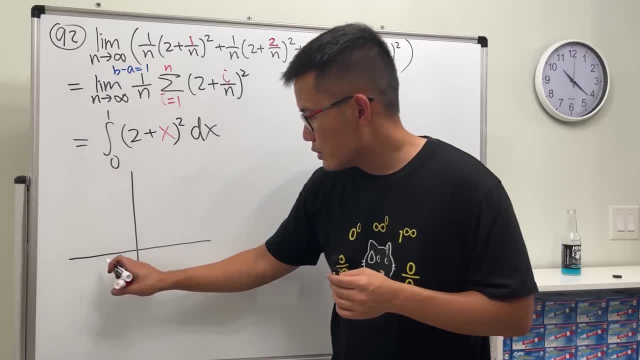 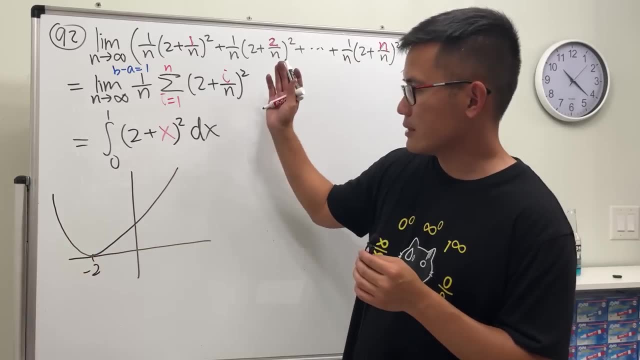 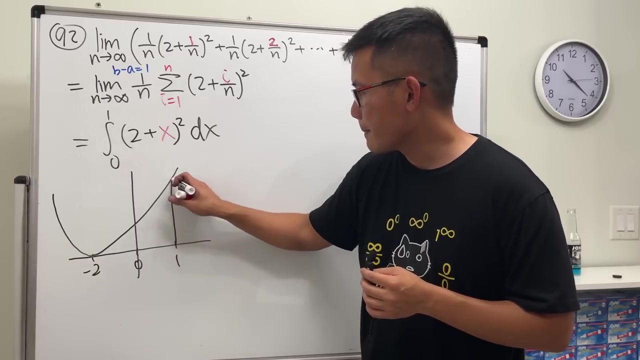 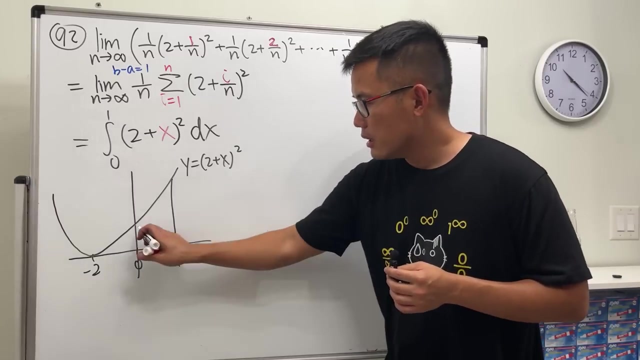 have a parabola, but you put to the left two units right, so when x is negative, 2, here we have a parabola something like this: okay, and i'm saying that the region that we want is from here to here is 0 to 1.. and then have a look, this is: y equals 2 plus x. oh, to the second power. does this satisfy? 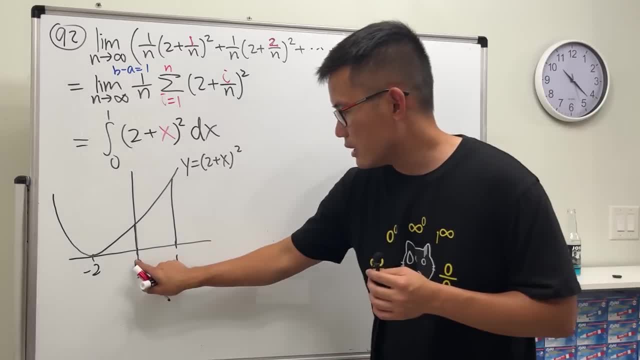 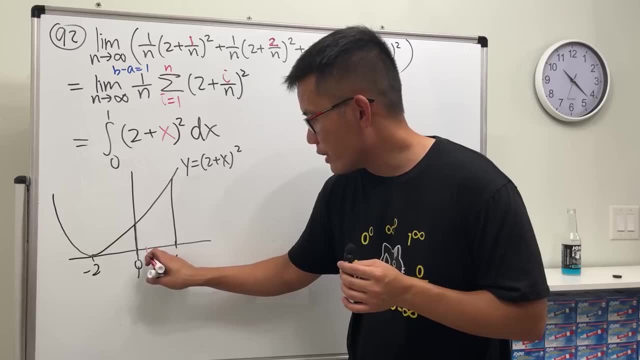 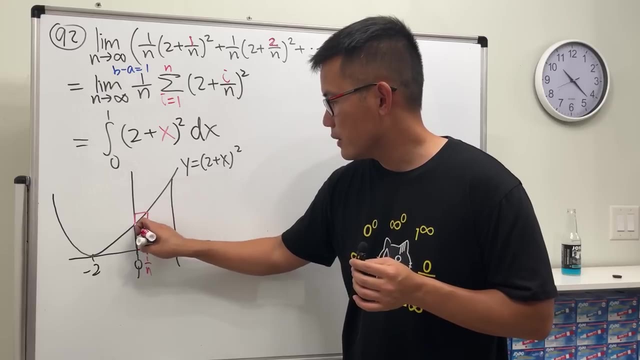 our original. it does have a look. we go from here to here. so the whole thing is 1 cut into n pieces. so each piece is 1 over n. so the first x value that we can use is 1 over n. put it here: the height is what? 1 over n in here. so 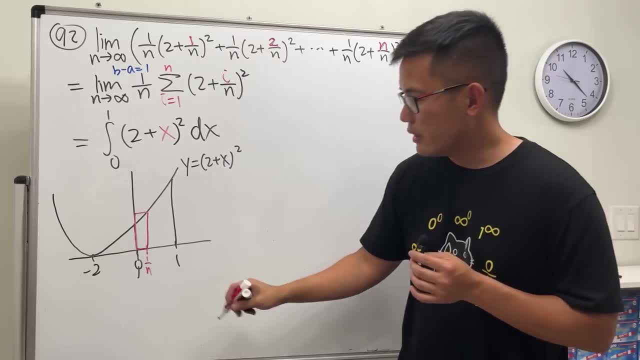 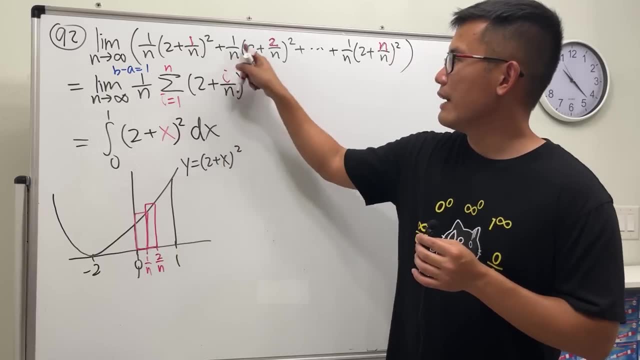 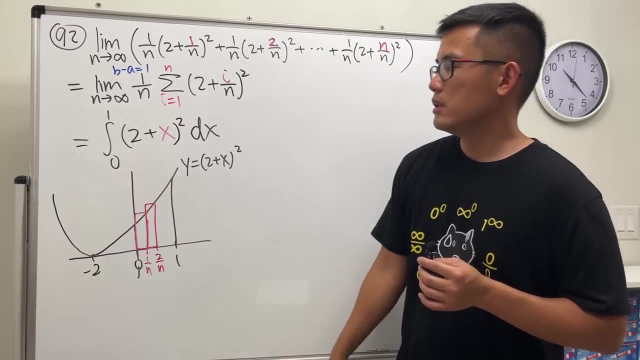 we have 2 plus 1 over n squared. the next x value 2 over n. put it here: we have 2 plus 2 over n squared. that's the height, and then everything. here the width is 1 over n. so yeah, let's convince you guys. 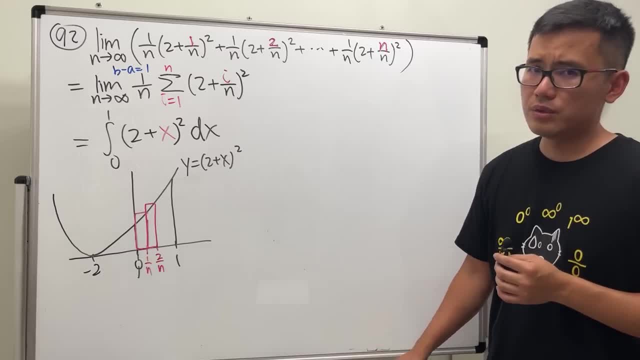 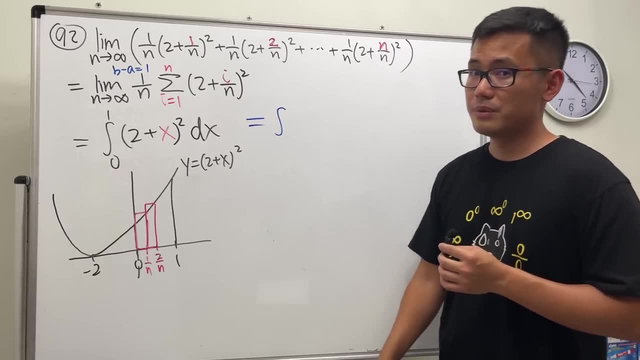 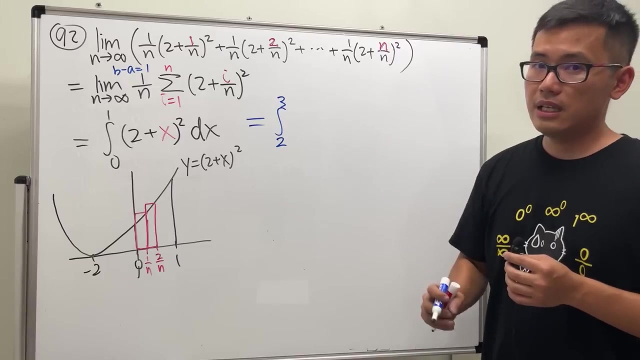 okay, what if you don't want to start with 0? i don't know. if you want to start with 2, it's okay too, i'll show you. if you start with 2, then you go up to 3 per our discussion earlier. right, and in that case, the function. 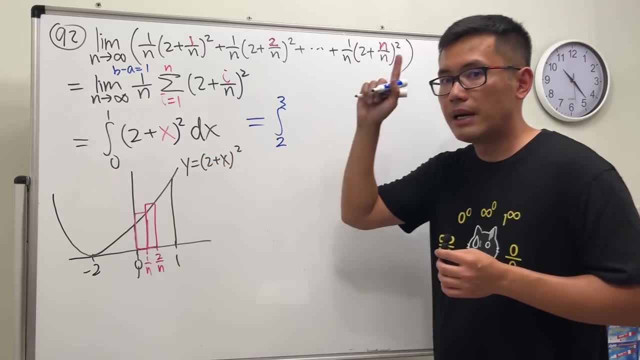 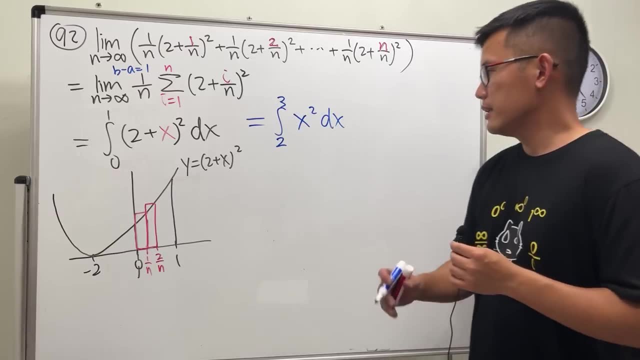 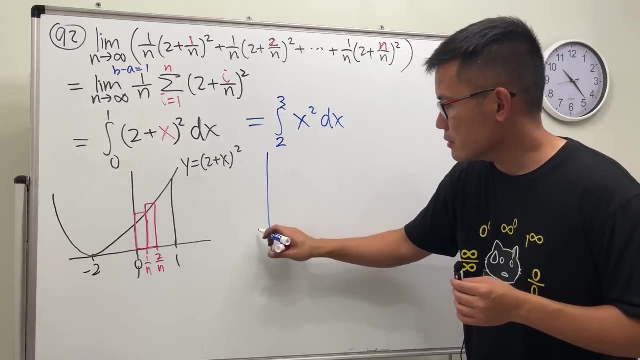 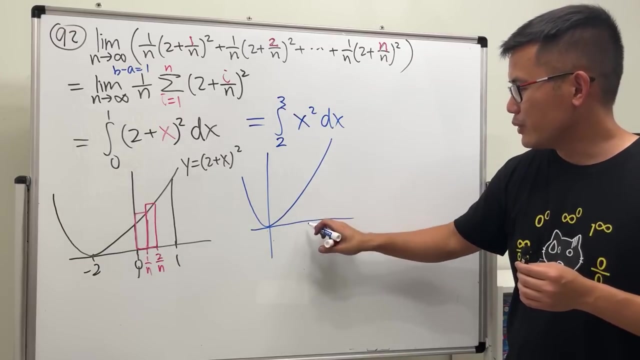 is no longer the same right here, but you put it as just x squared. why? let me show you this right here. will give you that as well. check this out. so we have our x square horrible picture. i know i'm sorry, but if we go from 2 to 3, so this is the. 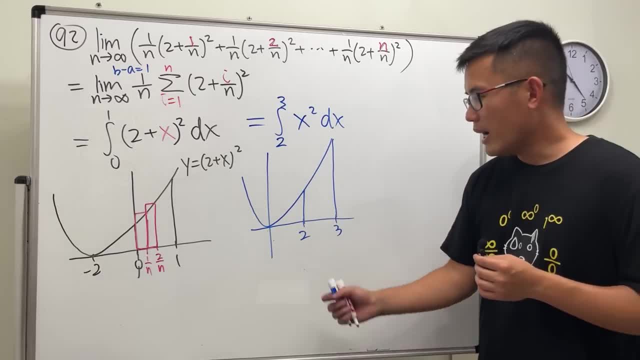 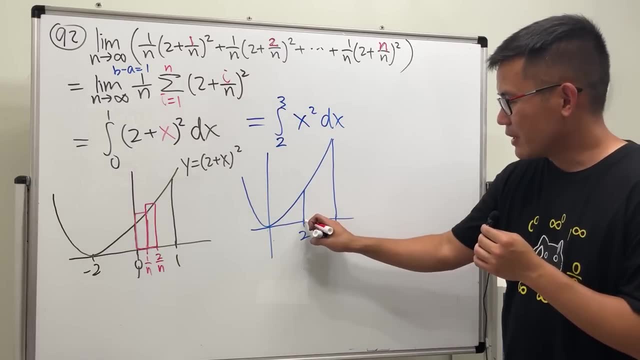 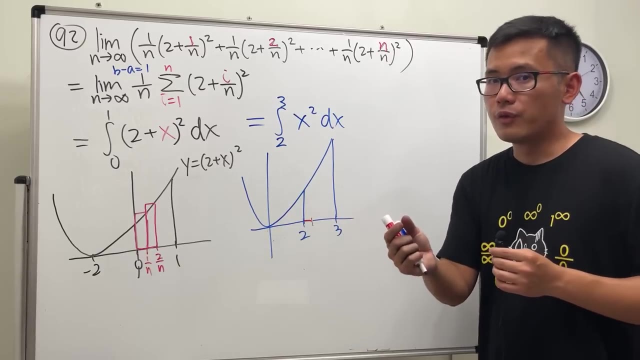 region that we are talking about now. okay, why we start with 2? because this right here is a 2. check this out: from here to here, the whole thing is still 1 cut into n pieces. so this right here the width is still 1 over n. 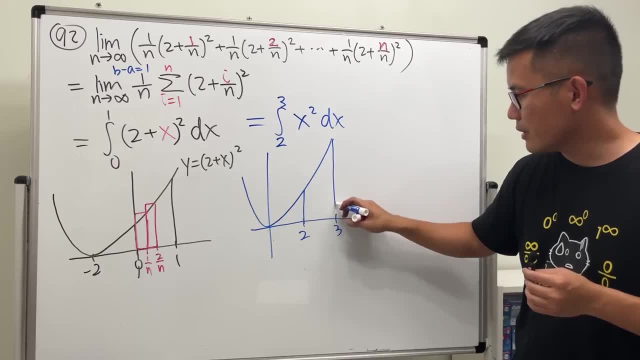 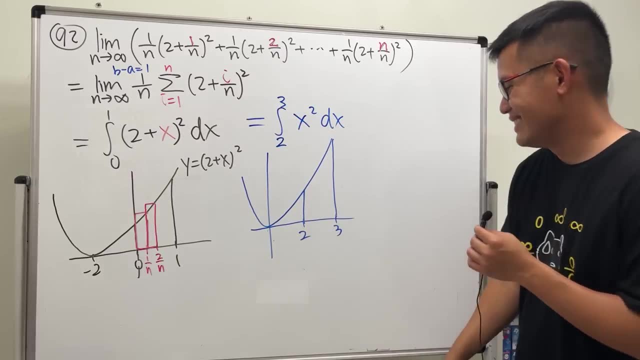 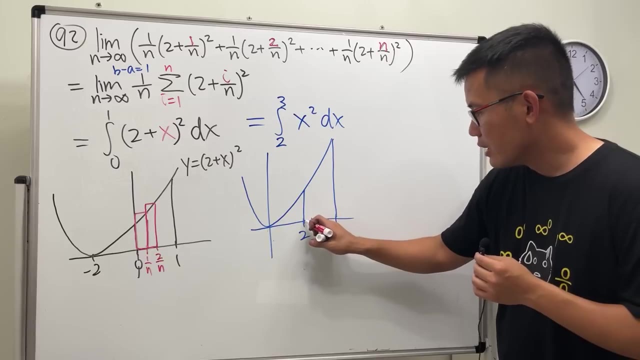 two to three. this is the region that we are talking about now. okay, why we start with two? because this right here is a two. check this out: from here to here, the whole thing is still one cut into n pieces. so this right here the width is still one over n. 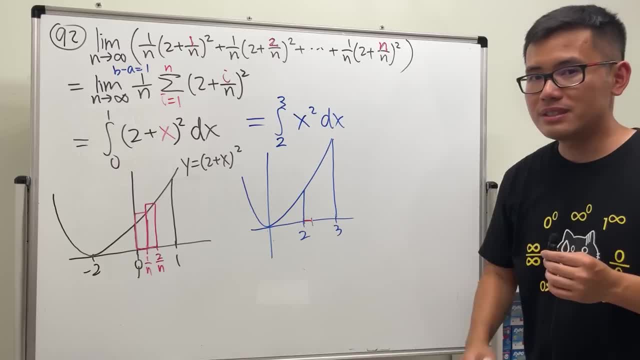 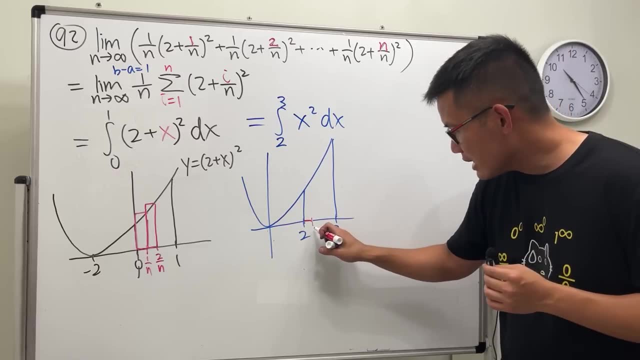 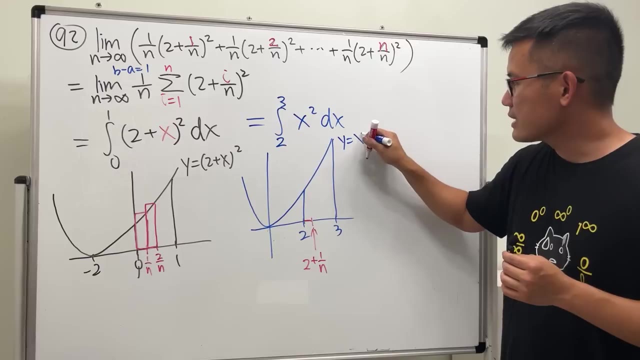 so we still have one over n there. good, but what's the x value from here to here is two. we have to add one over n, so this x value is two plus one over n, and then you see, our function is x squared. we are going to put this whole thing. 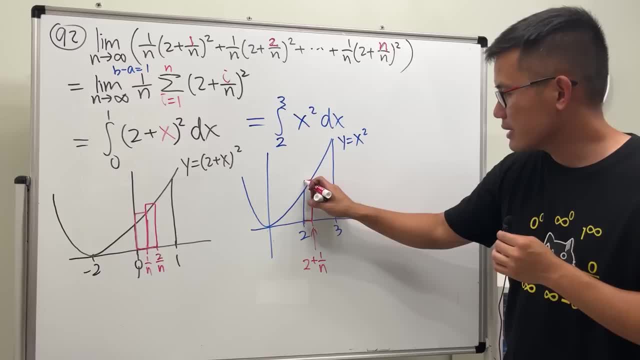 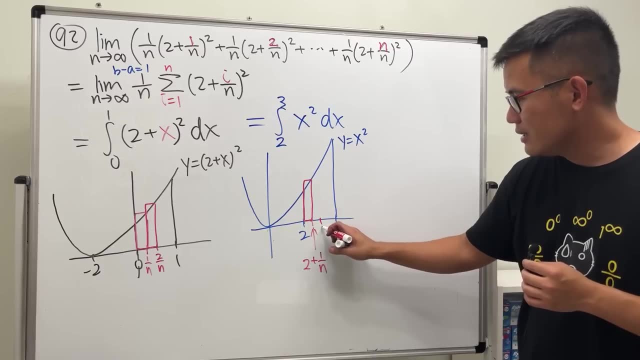 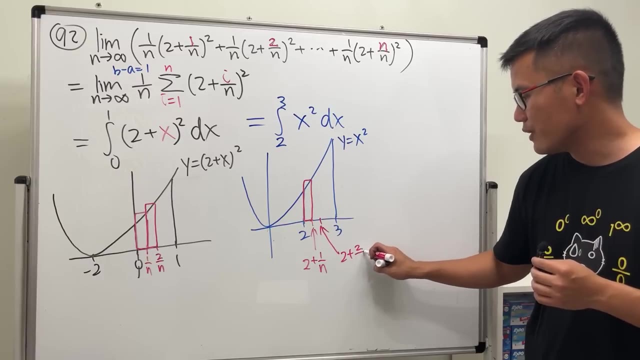 two plus one over n to here, and then go up. you see, that's how we get the height, which is that same thing. next, this right here, is what, from here to here, is two, one over n, another one over n. so all to get is two plus two over n. 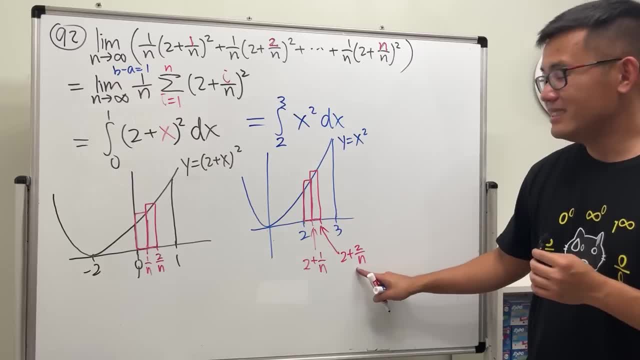 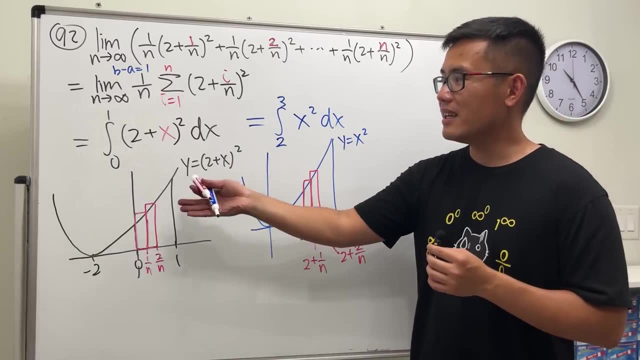 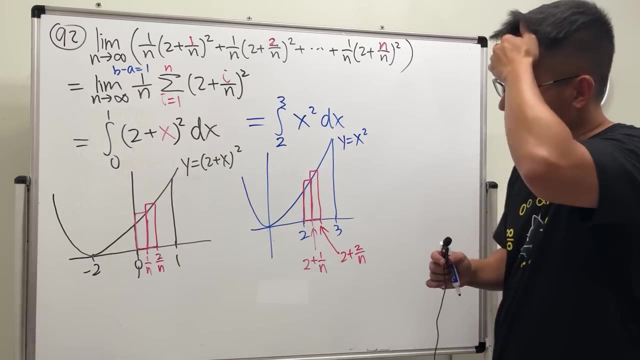 whoa, look at that. this is the x value. put it here. look at that same thing. so that's why, as I said, just always start with zero for this kind of equations. everybody will be so much happier. if you don't want to start with um, if you don't want to start with zero, 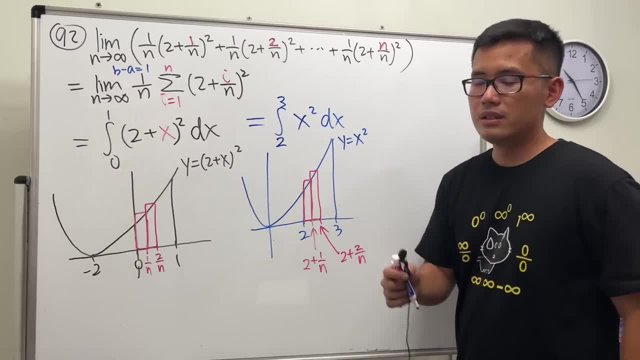 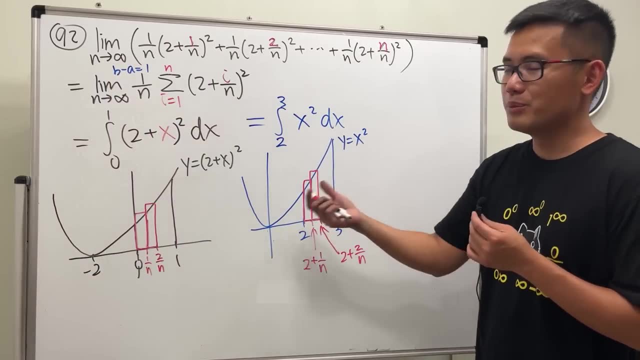 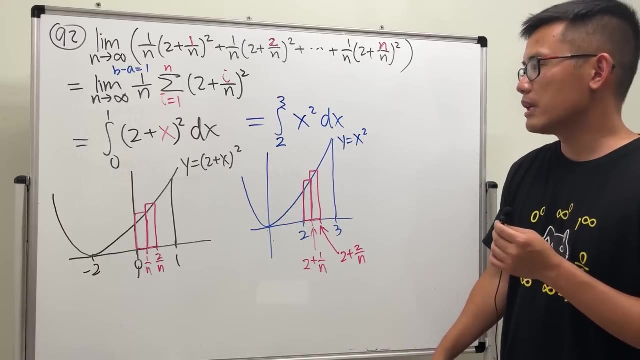 that's totally okay. it's just that you kind of move the region around. this is a microphone I move to here that still move the microphone- same thing. so it doesn't matter how you move it horizontally, you will still have the same area under the curve. it's easier to compute, though, so 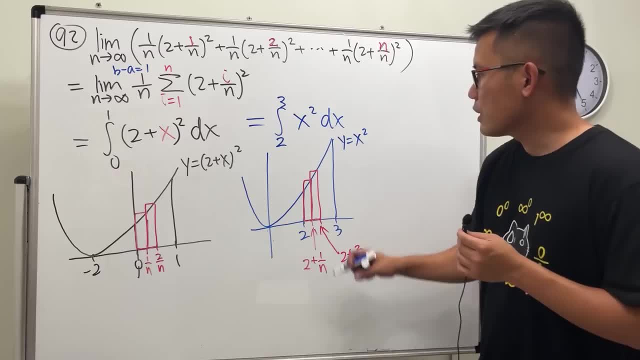 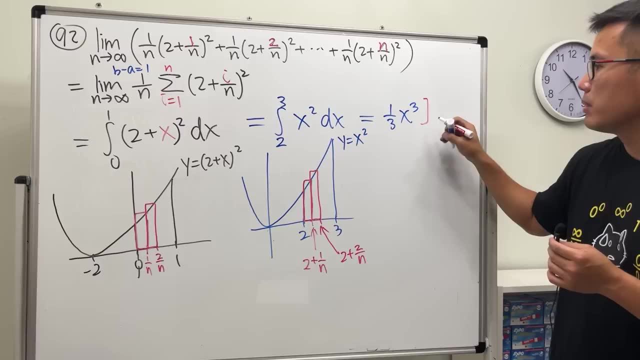 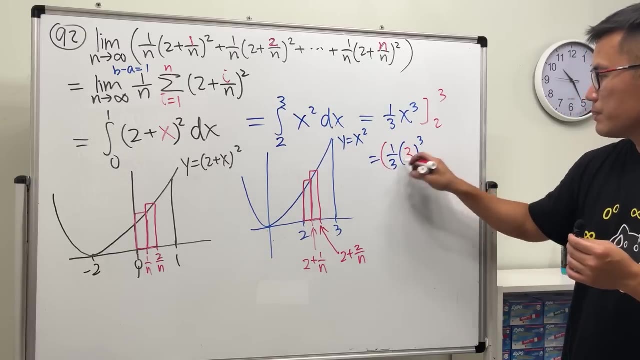 that's the advantage, alright, so I'm going to compute this for you guys. do the same thing, antiderivative. so you get one third x to the third power, and then we plug in two, three, this right here: one third three to the third power. that's the first part. 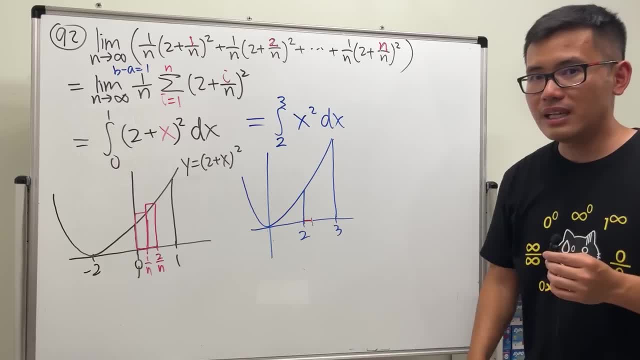 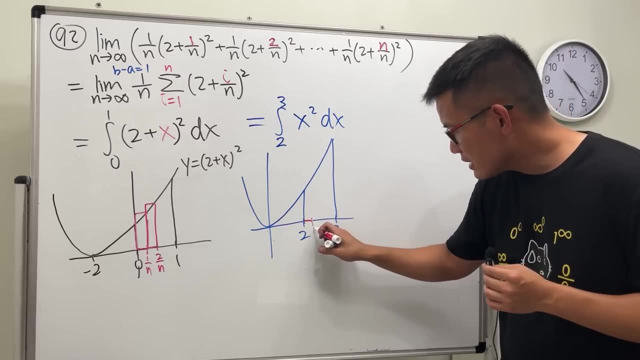 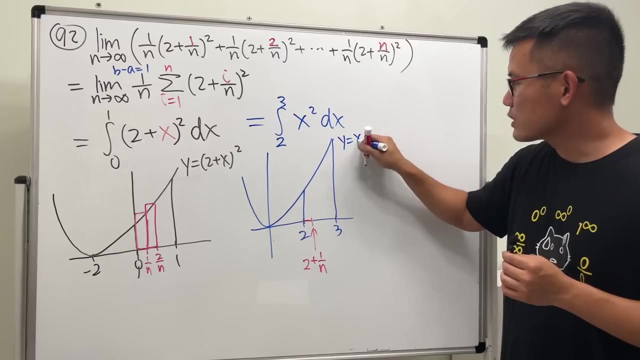 so we still have one over in there. good, but what's the x value from here to here is 2. we have to add 1 over n, so this x value is 2 plus 1 over n and then you see our function is x squared. we are going to put this whole thing- 2 plus 1 over n- to here and then go up. 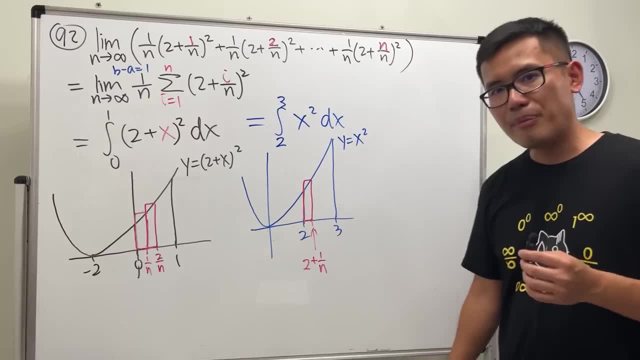 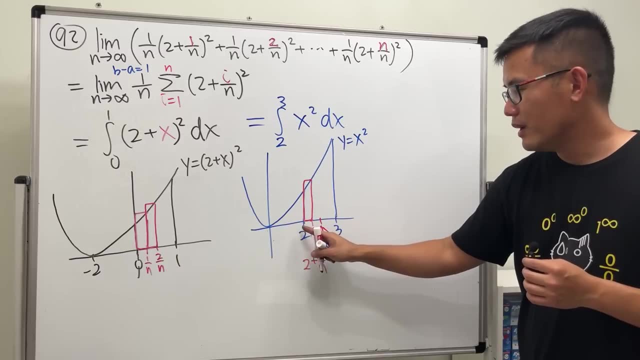 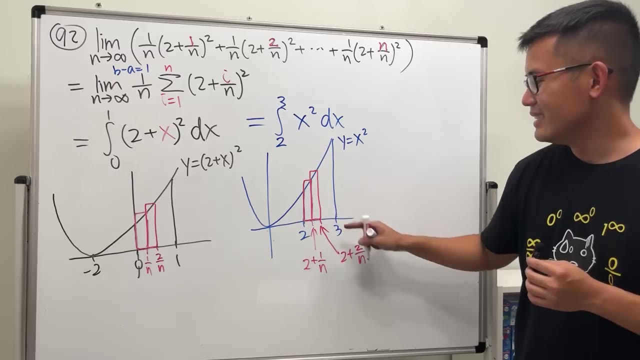 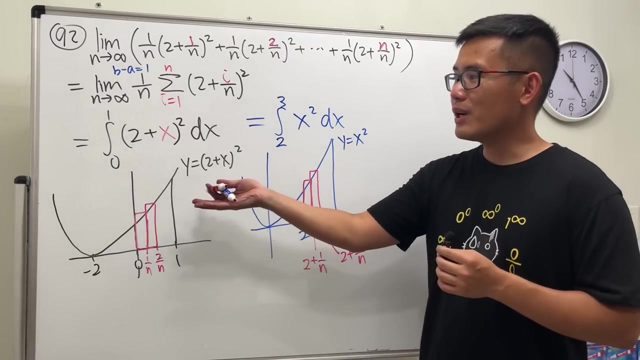 that's how we can get height, which is that same thing. next, yeah, this right here is what, from here to here, is two, one over n, another one over n. so all to get is two plus two over n. whoa, look at that. this is the x value. put it here. look at that same thing. so that's why, as i said, 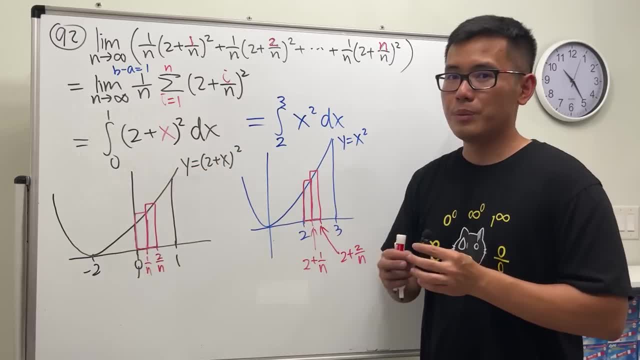 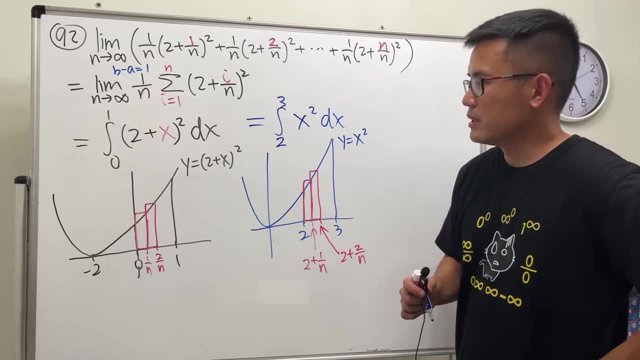 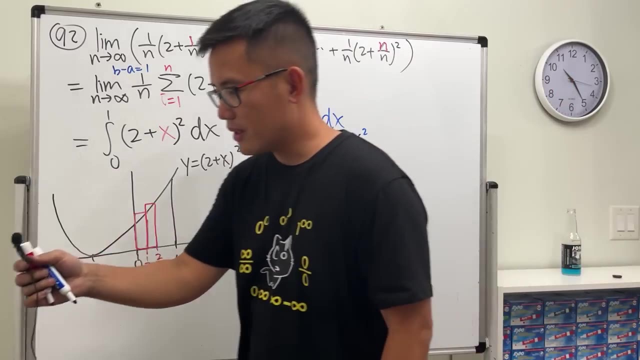 just always start with zero for this kind of questions. everybody will be so much happier. if you don't want to start with um, if you don't want to start with zero, that's totally okay. it's just that you kind of move the region around. this is a microphone i moved to here. let's still move. 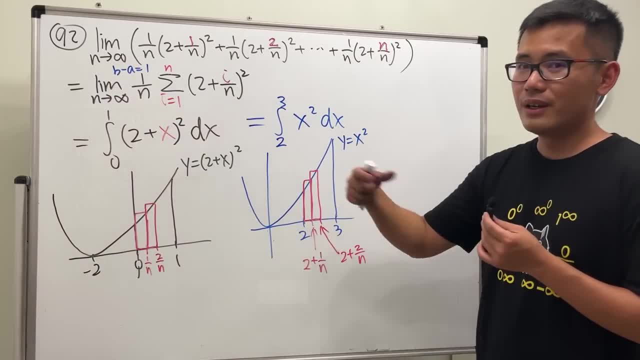 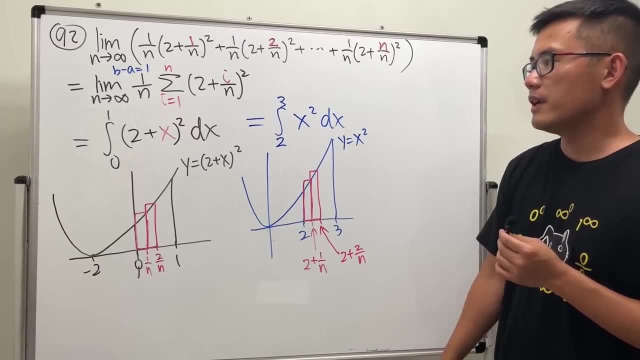 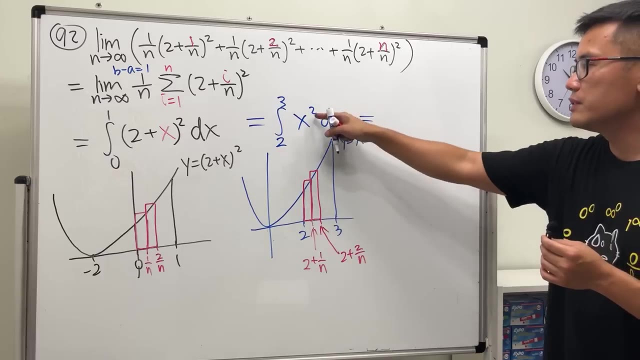 the microphone. same thing. so it doesn't matter how you move it horizontally, you will still have the same area under the curve. this right here is definitely easier to compute, so that's the advantage. all right, so i'm going to compute this for you guys. do the same thing, anti-derivative, so you get. 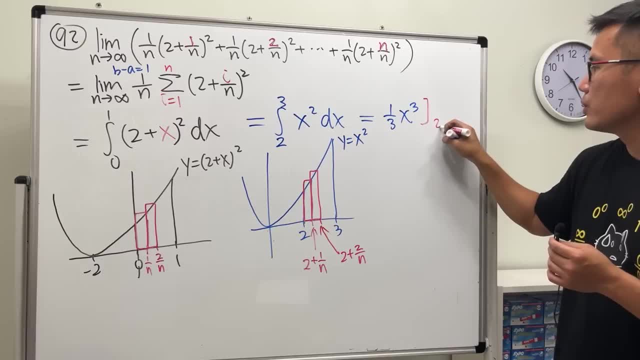 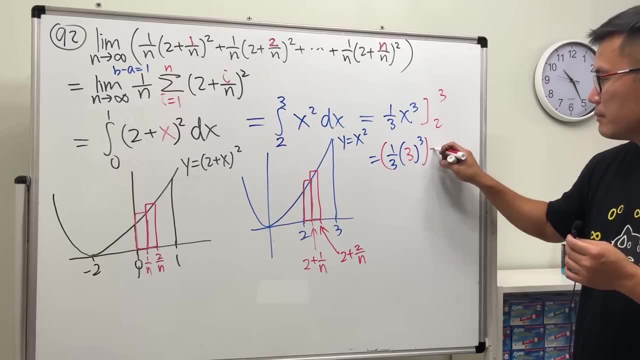 one third x to the third power, and then we plug in two, three. this right here: one third three to the third power. that's the first part, and then minus one third two to the third power. yeah, okay, that's 27, 27 minus nine. twenty seven minus nine. 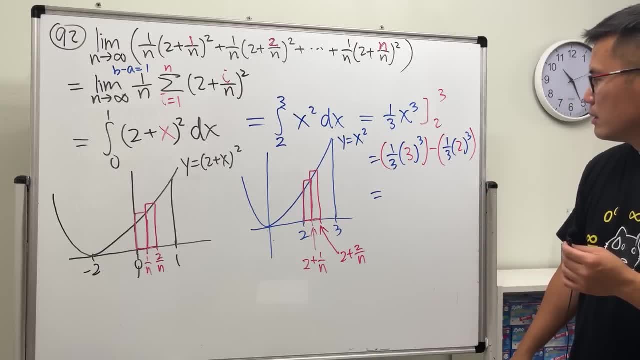 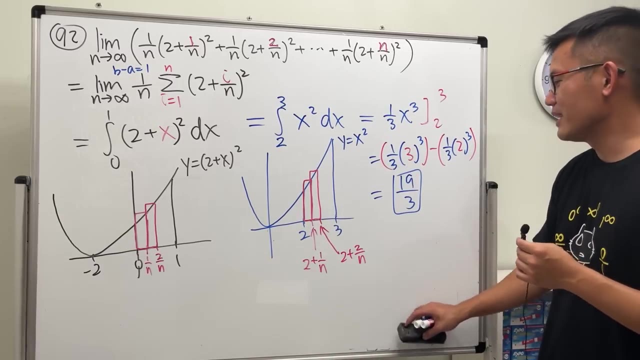 18.. no, that's eight. oh, my goodness. twenty seven minus eight, nineteen, right, twenty seven minus eight. this is this nineteen over three. there we go, almost starting right. i was saying, oh, how can this be so nice to be like three? not possible. if you do this, you get the same answer. 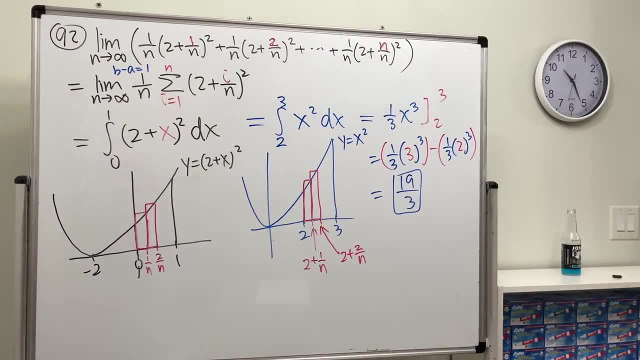 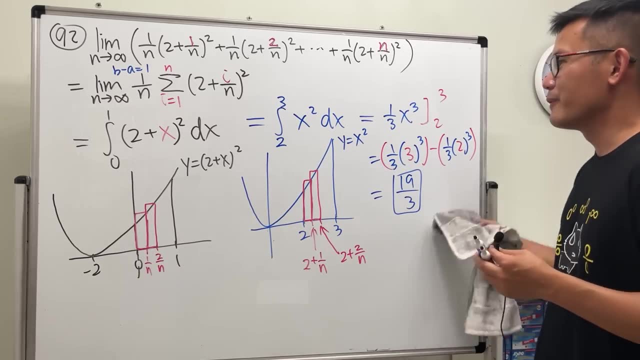 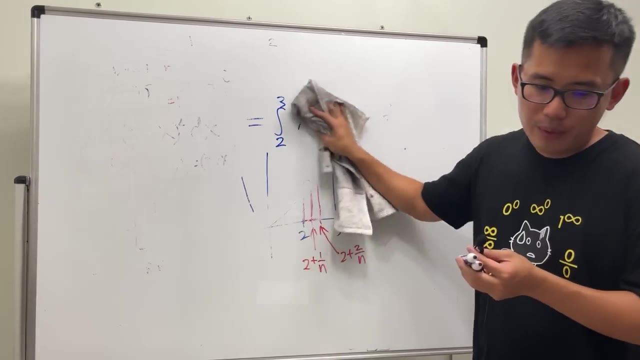 all right, let me see if the okay. yes, my phone is recording almost seven hours. oh my god. i thought i was able to finish this in six, but no, all right. so, with that being said, i'm just going to show you guys how we can quickly set all this up and then, if necessary, i'll show the pictures. 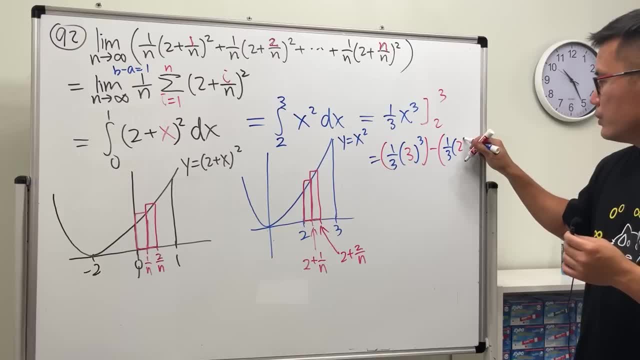 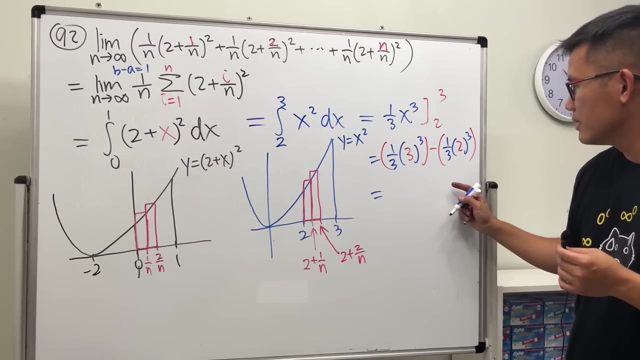 and then minus one third, two to the third power. yeah, okay, that's twenty seven. twenty seven minus nine. twenty seven minus nine. twenty seven minus nine, eighteen, eighteen, no, that's eight. oh my goodness. twenty seven minus eight, nineteen, right. twenty seven minus eight. this is nineteen over three. there we go. 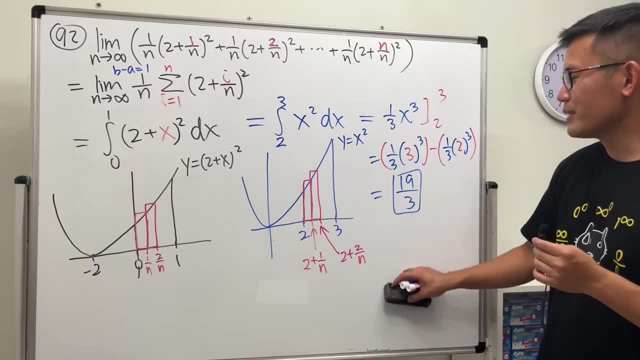 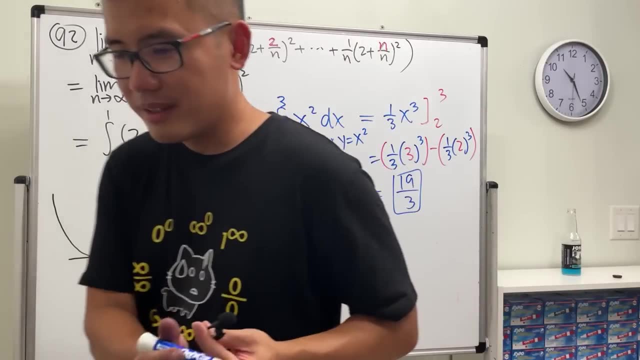 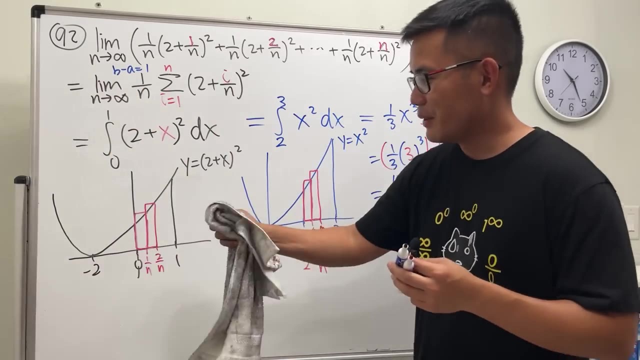 almost got it right. I was like: how can this be so nice to be like three, not possible. if you do this, you get the same answer. all right, let me see if the okay. yes, my phone is recording almost seven hours. oh my god, i thought i was able to finish this in six, but no, all right. 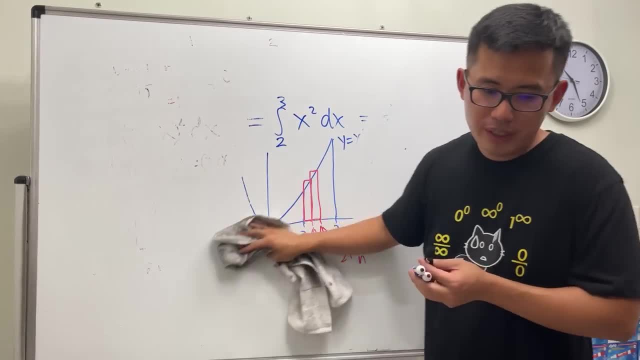 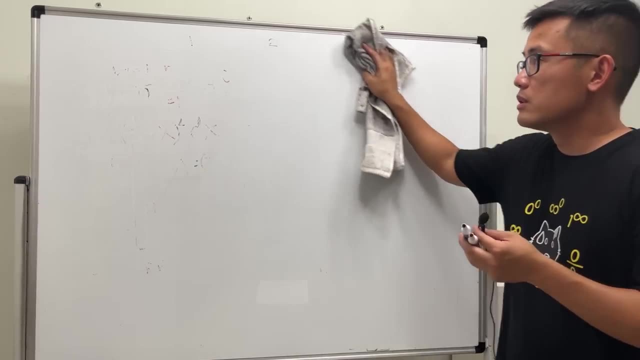 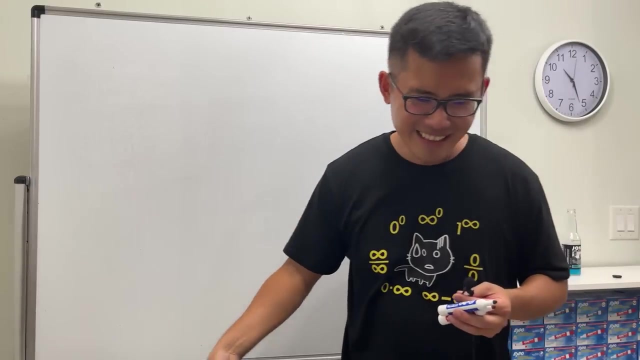 so, with that being said, i'm just going to show you guys how we can quickly set all this up, and then, if necessary, i'll show the pictures to convince you guys that it's actually correct, and then, um, we'll do the integrals, and then that's it. that's it, number 93. oh, my god, number 93. 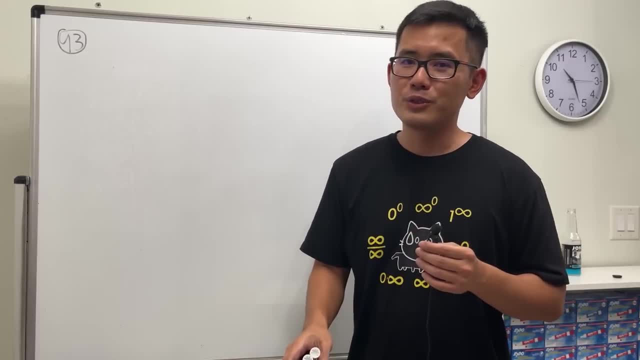 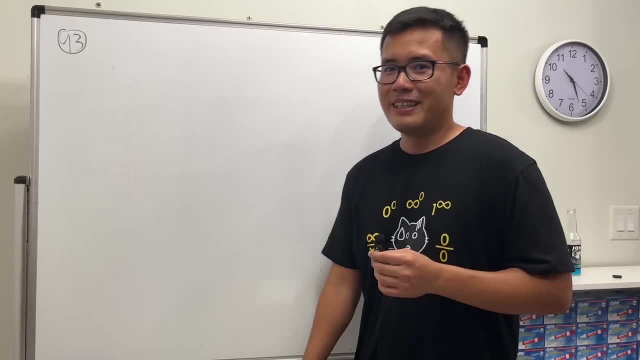 yeah, i want to thank everybody, though, whoever is still watching right now. thank you guys so much. i want to thank all my subscribers, all my channel members, all my patrons. thank you guys so so, so much. almost 1 million subscribers still. thank you guys so much. thank you guys so much. thank you guys so much. 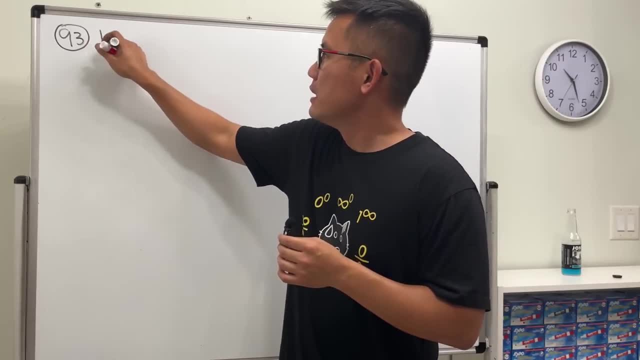 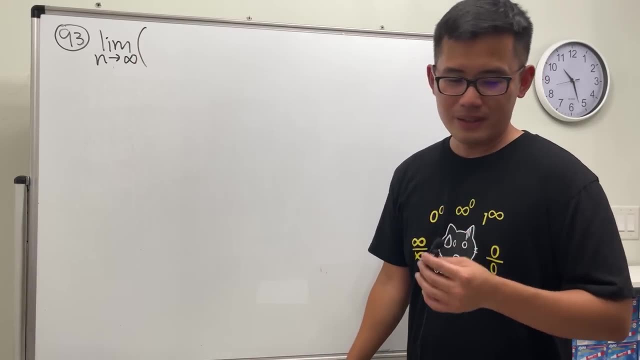 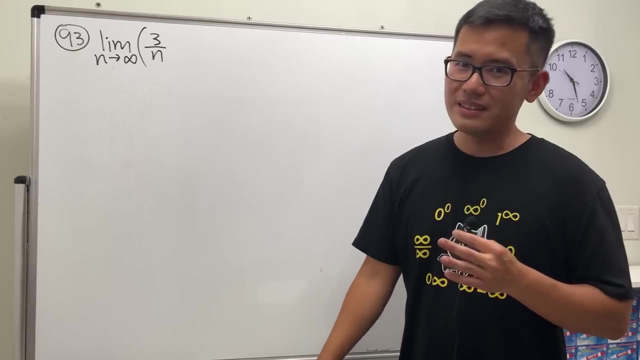 93. limit as an approach and infinity. it's just so much fun to do math questions um, and then you guys are watching and participating and giving your thoughts and all that stuff. it's also so much fun. love you so much. and it's a lot of fun to do 100 questions in one go. 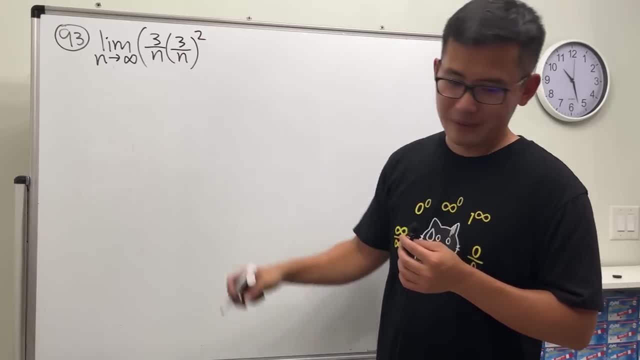 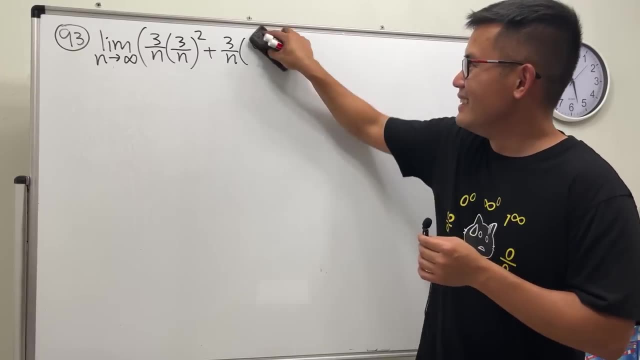 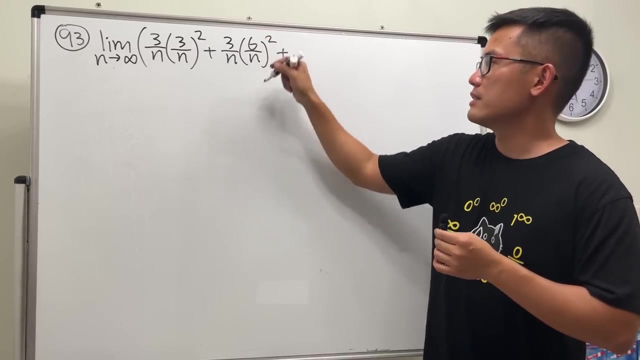 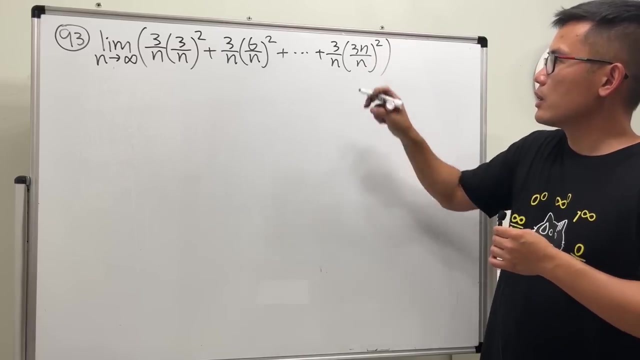 why? well, i don't have my reasons. so, yeah, same idea, but i'm hungry right now, so let me just finish. all right, six over n- square. the next one will be nine over n. okay, inside, and then cool. now put this in the sigma summation form. here we have the limit. 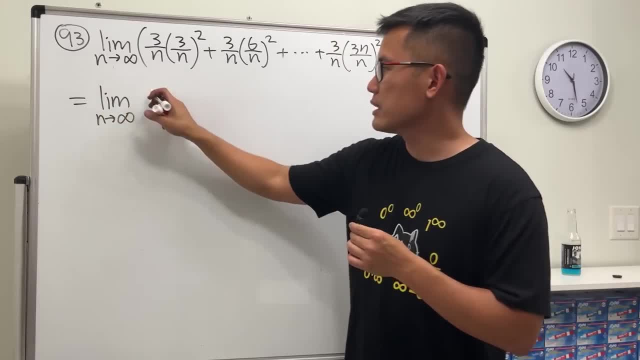 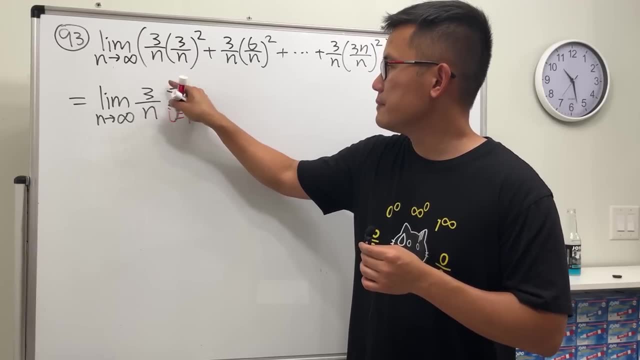 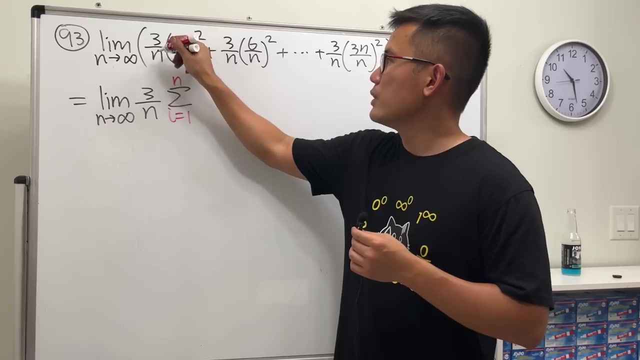 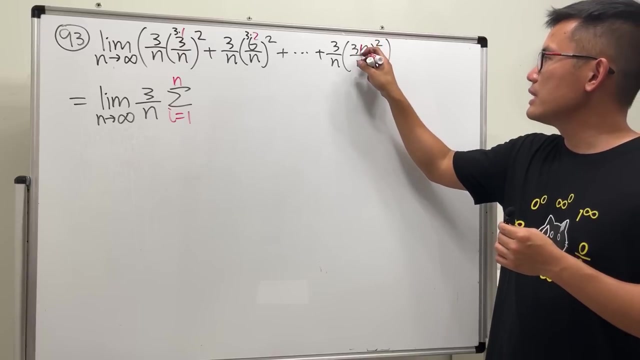 as n goes to infinity, everybody has three over n. so that's right. right here, sigma, i goes from one to n. i want to see one, two, three, four, all the way to n. so you do this. this is the same as three times one, this is the same as three times two, so on, so on, so on, and here we have three times. 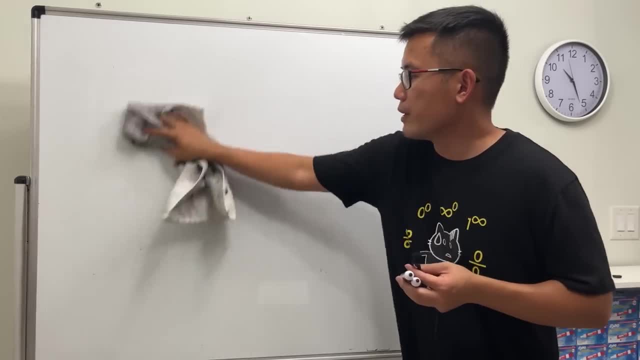 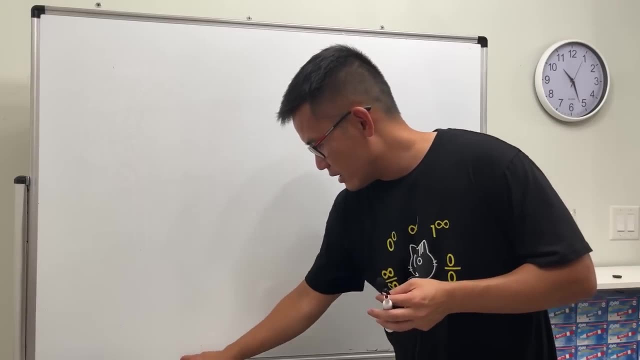 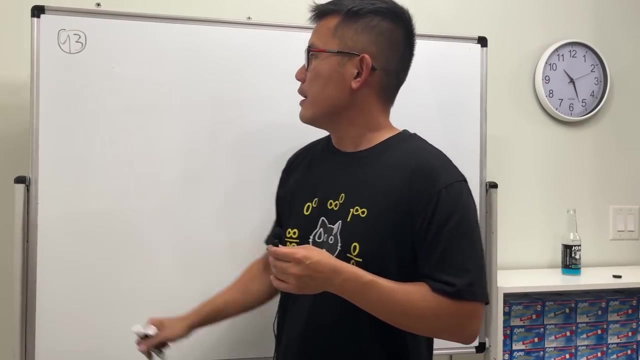 to convince you guys that it's actually correct, and then, um, we'll do the integrals and then that's it. that's it, number 93.. oh, my god, number 93.. yeah, i want to thank everybody, though whoever is still watching right now. thank you guys, so much. 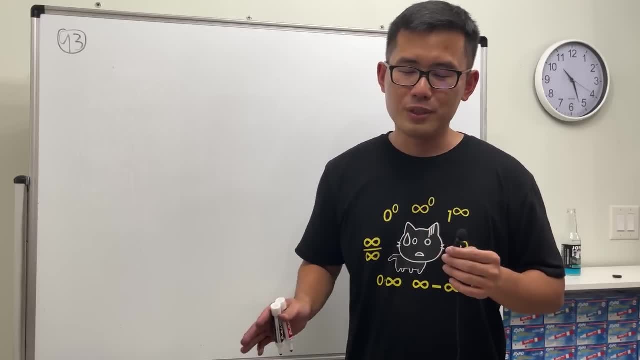 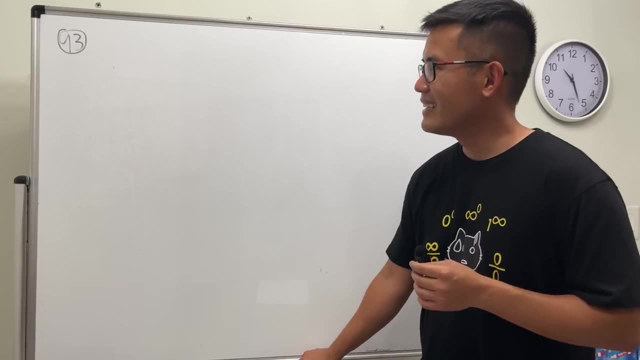 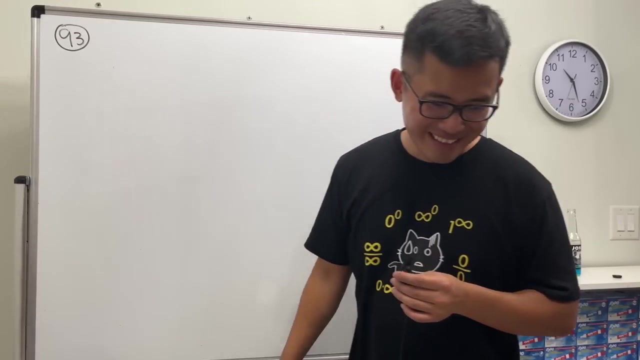 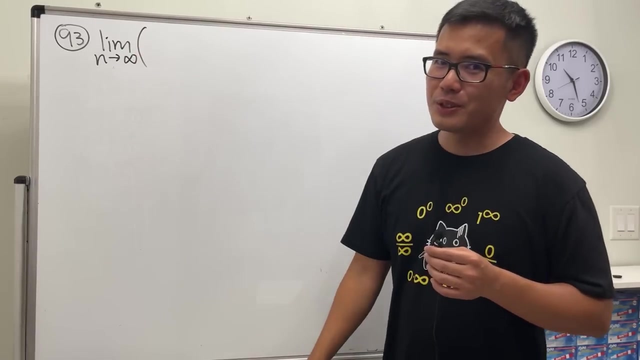 i want to thank all my subscribers, all my channel members, all my patrons. thank you guys. so so, so much. almost 1 million subscribers still. thank you guys, so much, so much. 93. limit as an approaching infinity. it's just so much fun to do math questions. 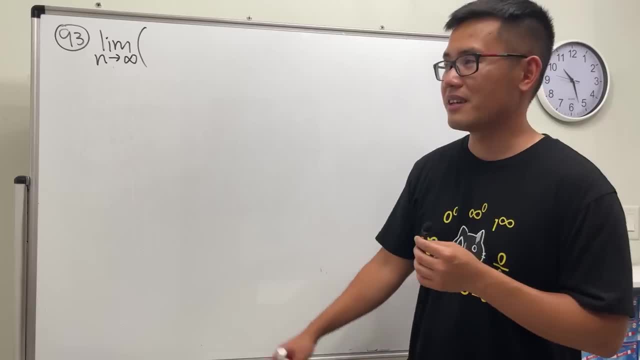 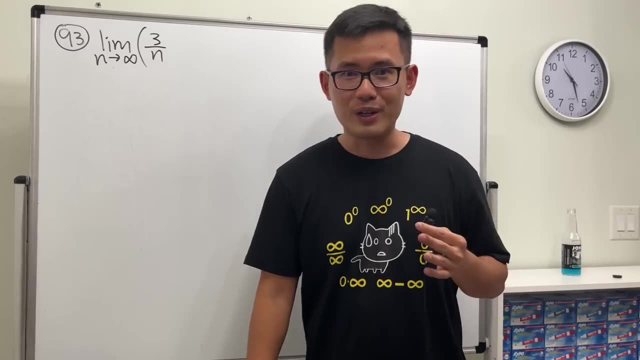 and then you guys are watching and participating and give me your thoughts and all that stuff. it's also so much fun. love you so much. and it's a lot of fun to do 100 questions in one go. why? well, i don't have my reasons. so 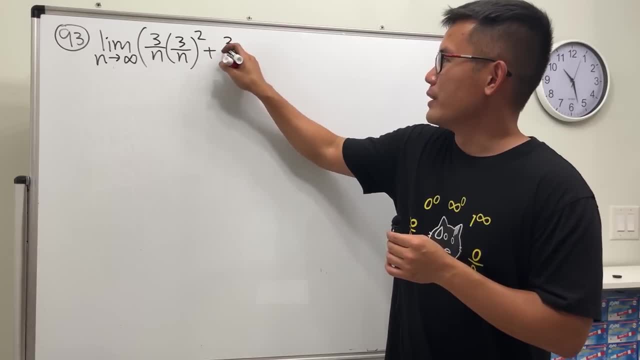 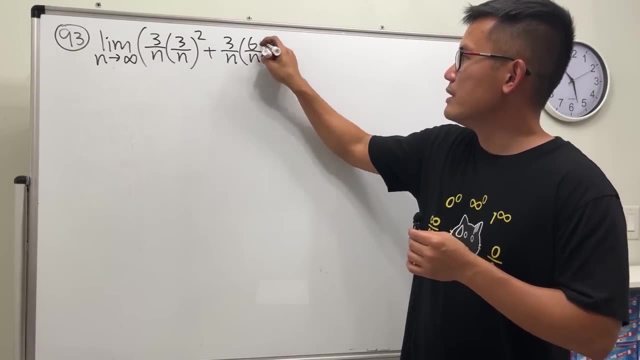 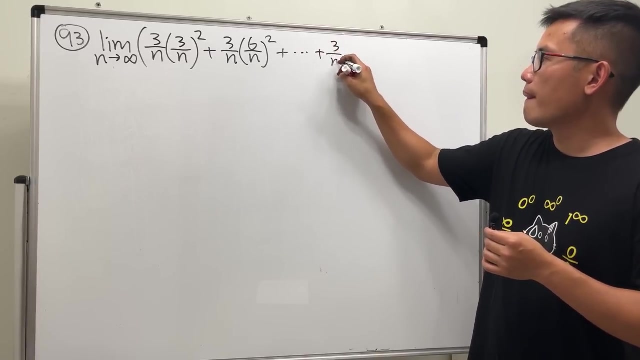 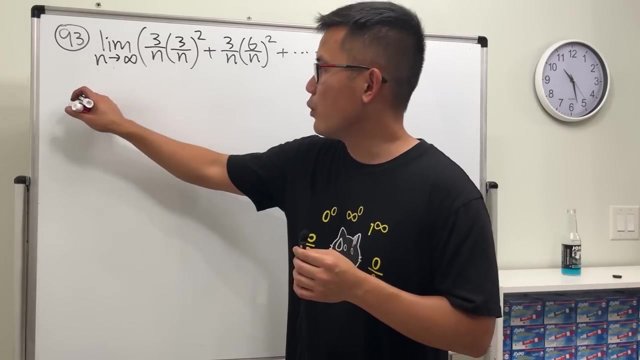 yeah, same idea, but i'm hungry right now, so let me just finish. all right, six over n- square. the next one will be nine over n. okay, inside, and then? cool. now put this in the single summation form. here we have the limit, as n goes to infinity. 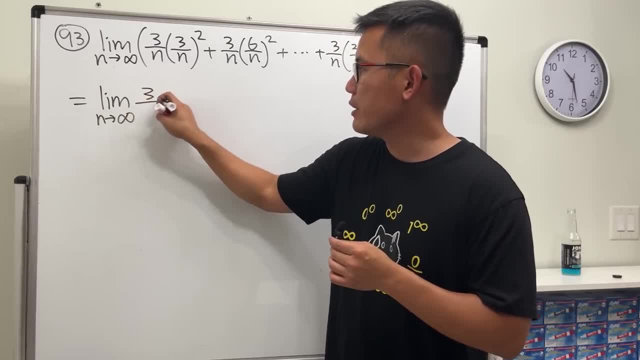 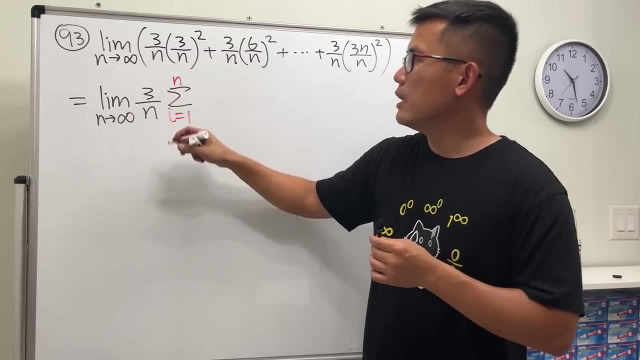 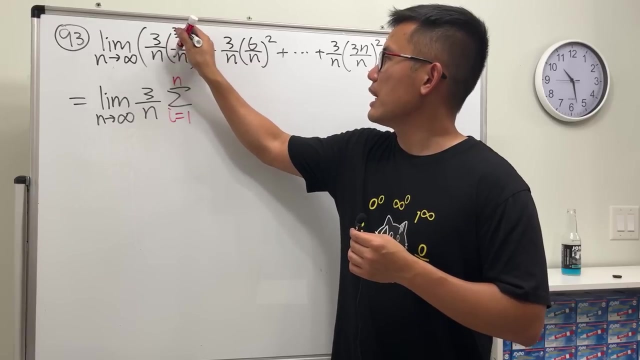 everybody has three over n. yes, that's correct. so that's right. it right here. sigma, i goes from one to n. i want to see one, two, three, four, all the way to n. so you do this. this is the same as three times one, this is the same as three times two, so on, so on, so on, and here we have three times n. 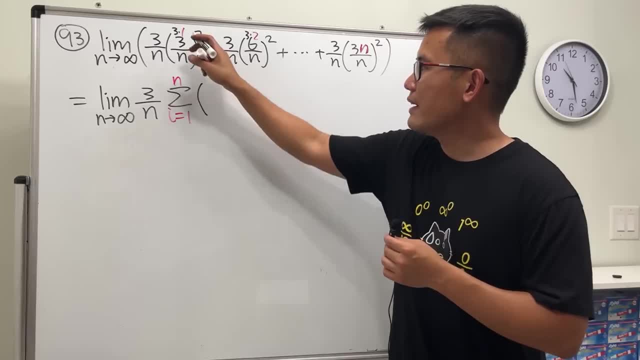 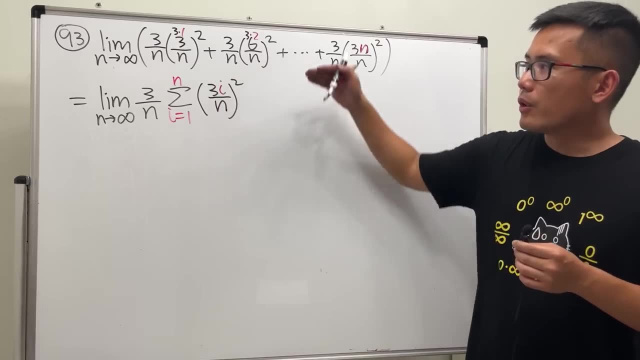 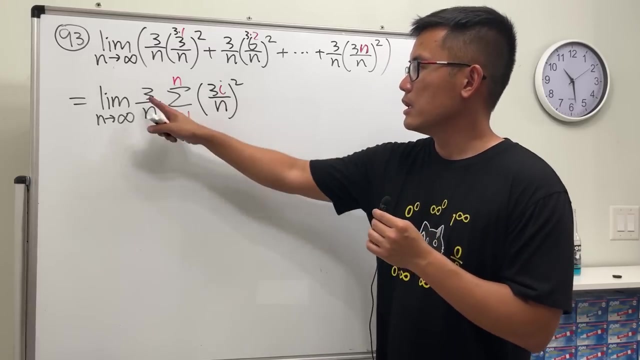 right, so that's the part that's changing. so we have three: i over n and then square. so the question can be presented this way or this way, so be careful with both ways. and here's an important point: you see, the three as you match. it's crucial, you'll see. but anyway, though, let's. 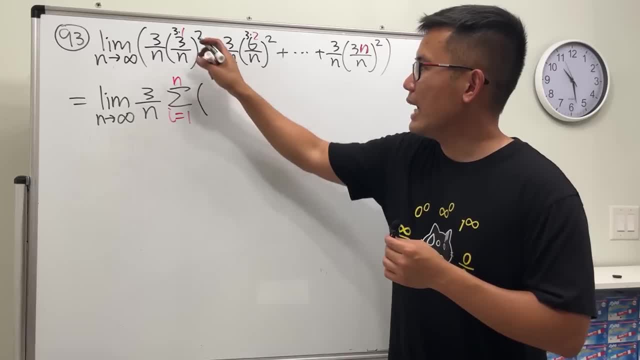 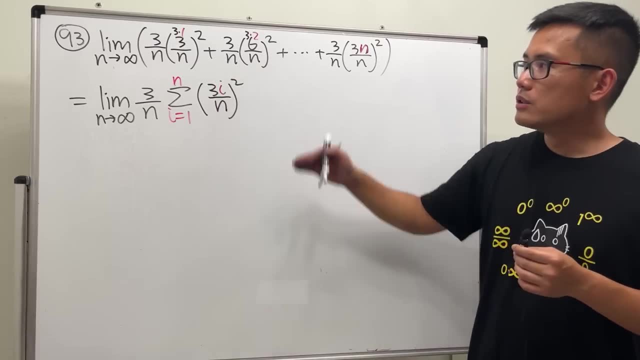 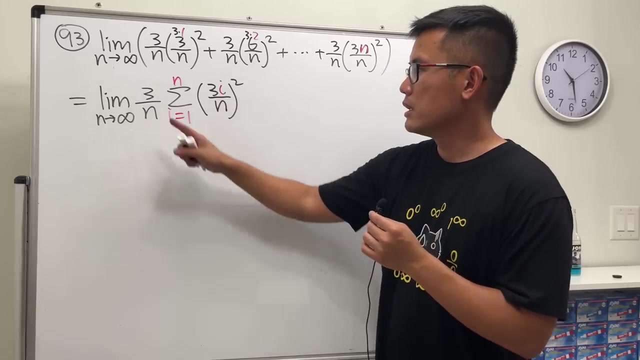 n, right, so that's the part that's changing. so we have three: i over n and then square. so the question can be presented this way or this way, so be careful with both ways. and here's an important point: you see the three as you match. it's crucial. 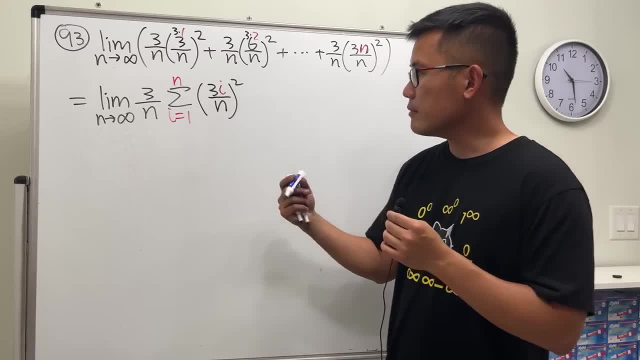 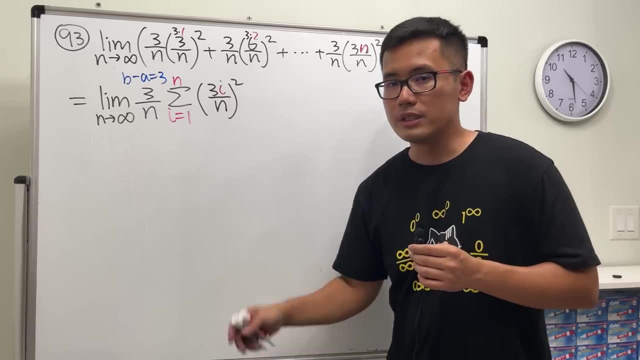 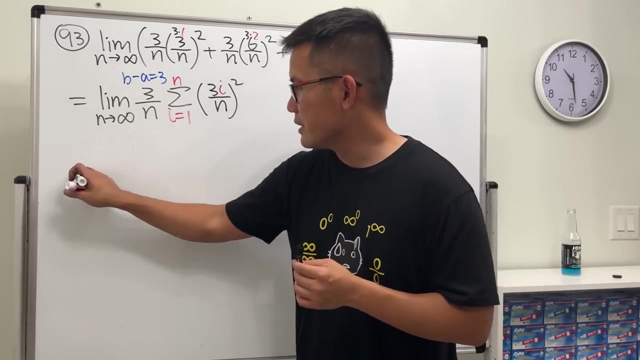 you'll see, but anyway though, let's do what we did earlier: three over n. this three tells us: b minus a is equal to three. so if we start with five, we go to eight. if we start with zero- which you should always start with zero- you go to three. so here's the deal: integral, zero to three. perfect, now what's? 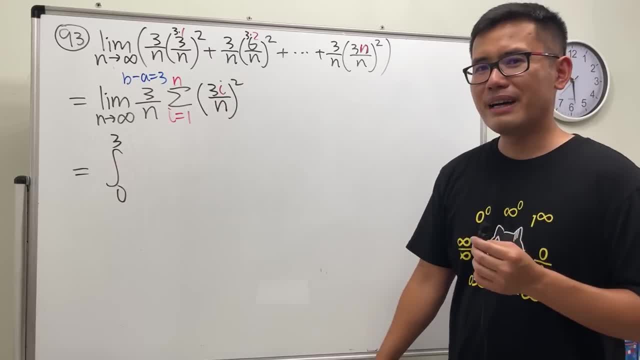 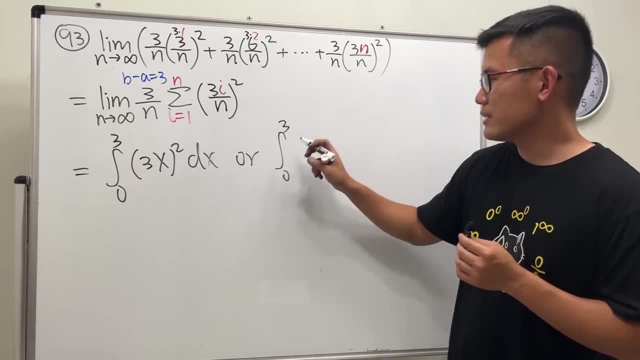 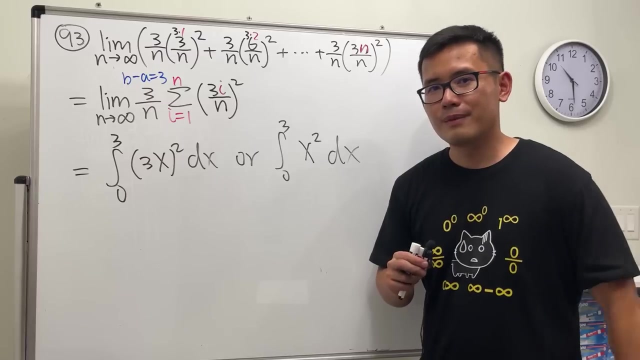 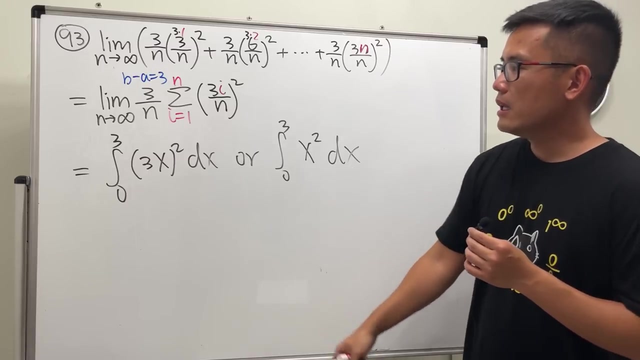 the function. we have a three right here. that's bothering us. is the function three x square or are we having just like zero to three x square, dx which one? the answer is this right here. not that this right here. why? because the reason that we have a studio right. 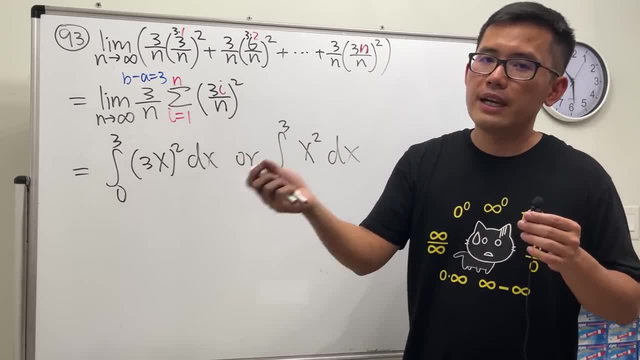 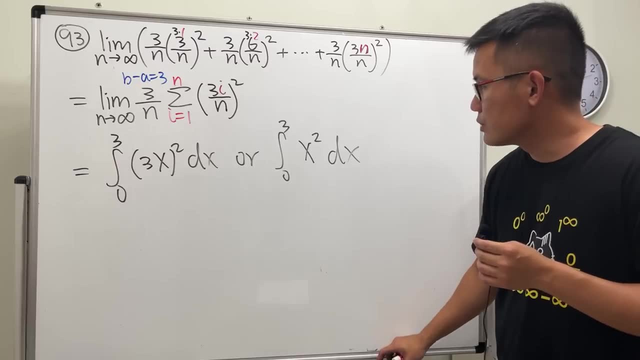 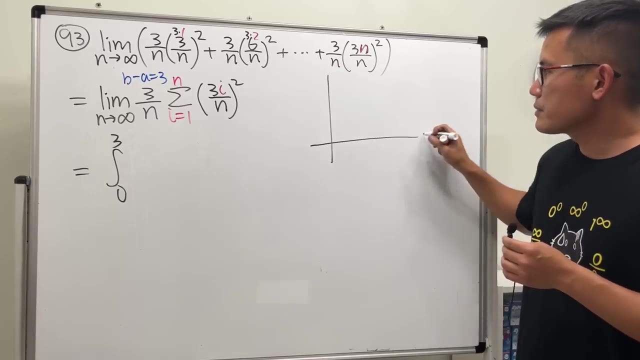 here is because the whole thing is three and we kind of end pieces. so that's why, and uh, i'm going to perhaps just erase this and i'm going to just give you guys a picture right here real quick. so you see, when we have uh, x to the some power, but it's actually just x to the 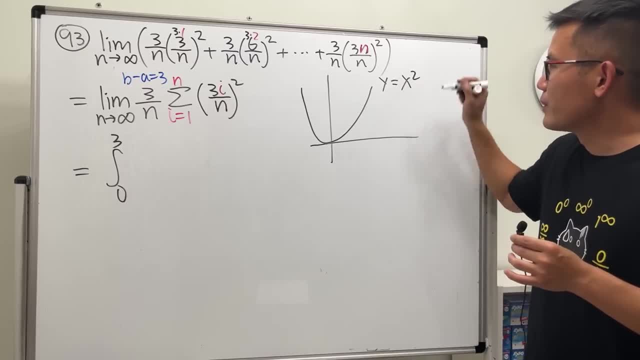 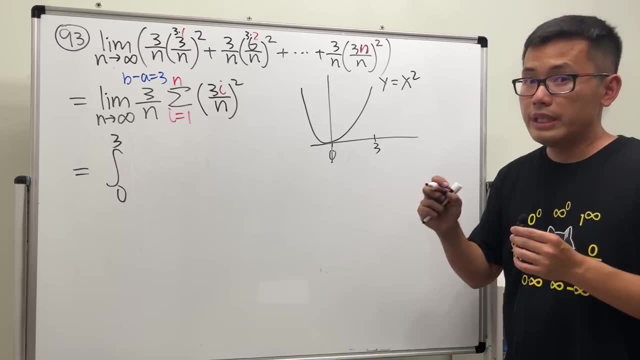 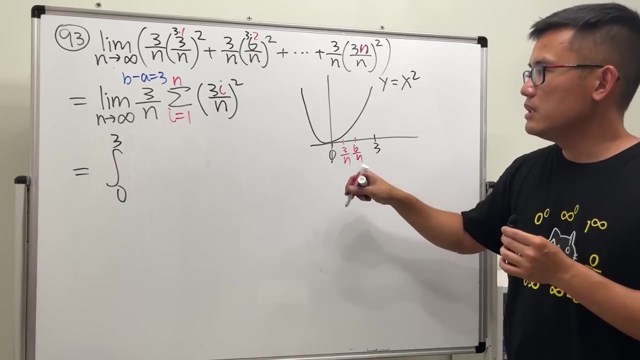 third power. but no, no, no, no kidding, just kidding x to a second power, because we're going from zero to three, right, so each width is three over n, the next one is six over n. so you see, that's why i said: students, you match. so you see, you put this. 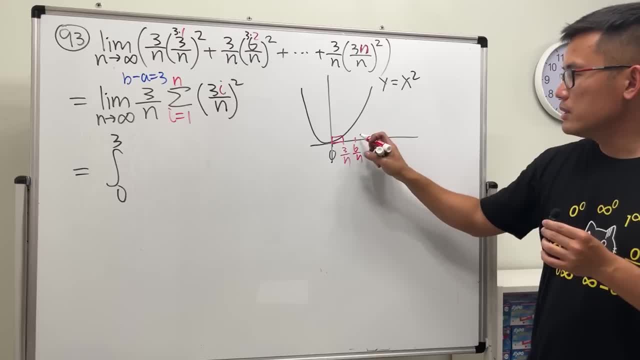 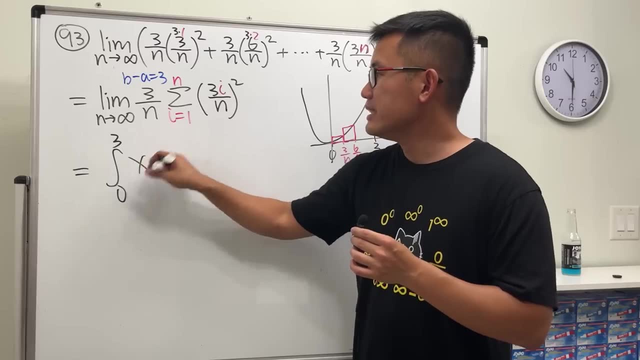 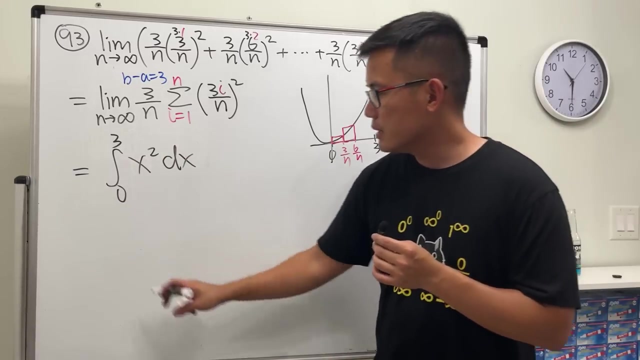 to the x value. we get that for the height. you put this to be x for you in. here you get the height. so the function is actually just x squared, it's not 3x squared. be really careful. so it's x squared- x. work that out. 1 third x to the third power: 0 to 3. 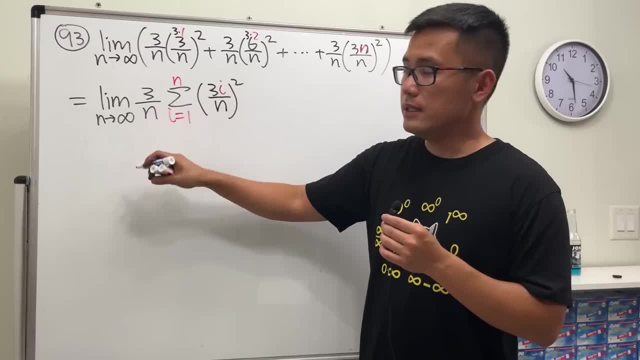 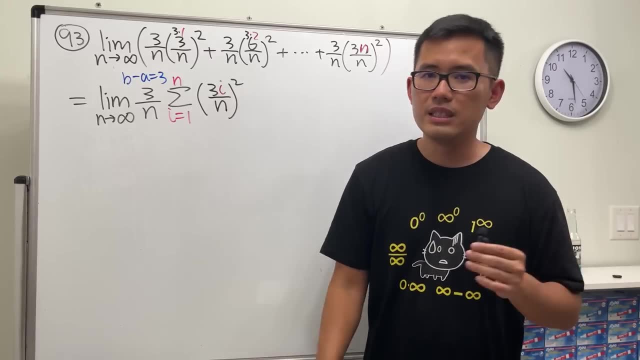 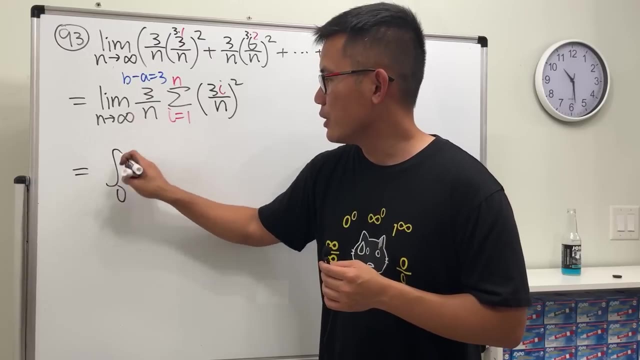 do what we did earlier: three over n. this three tells us: b minus a is equal to three. so if we start with five, we go to eight. if we start with zero- which you should always start with zero- you go to three. so here's the deal: integral zero to three. perfect, now what's the function? 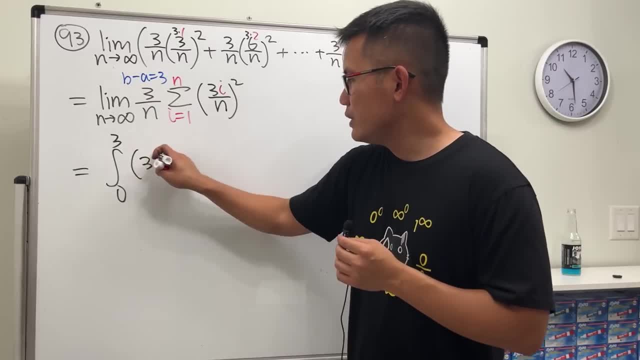 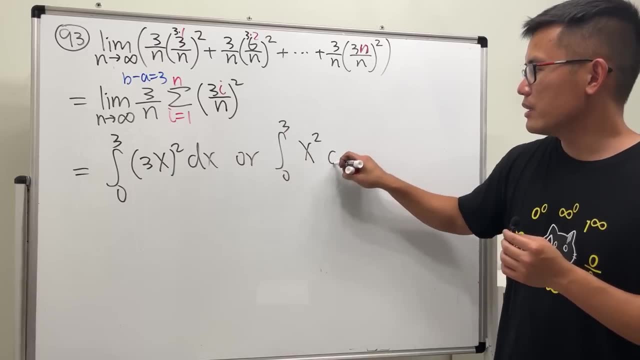 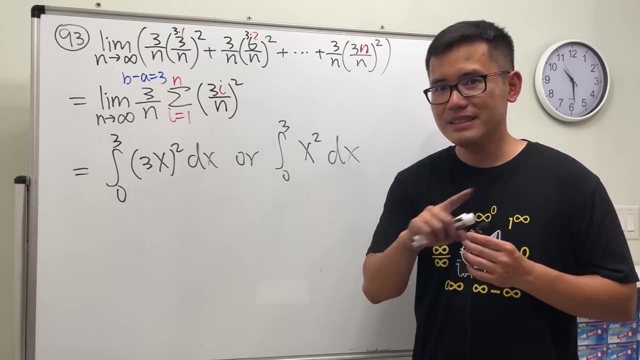 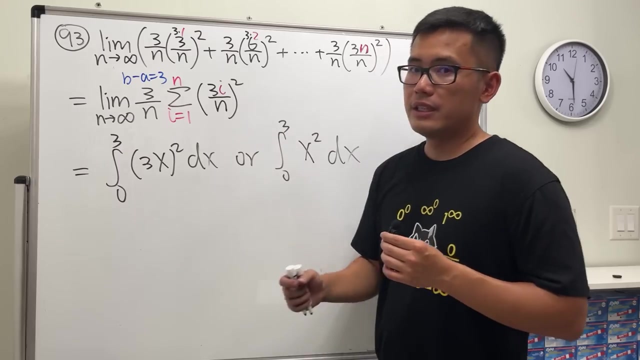 we have a three right here. that's bothering us. is the function three x square or are we having just like zero to three x square, dx which one? the answer is this right here. not that this right here. why? because the reason that we have a studio right here is because the whole thing is three and we cut into n pieces, so that's why. 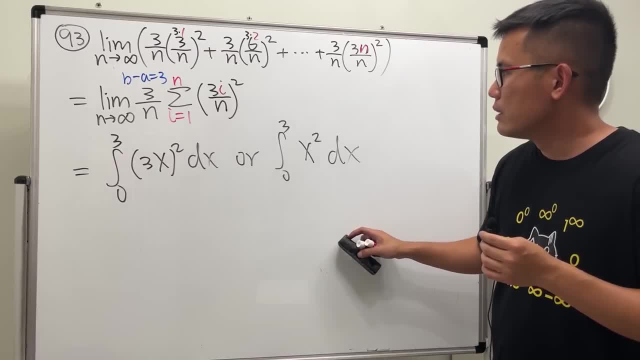 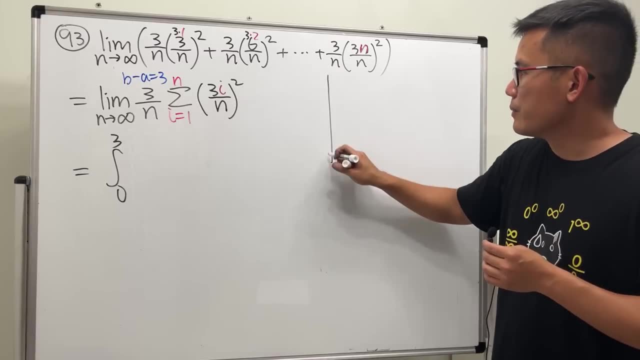 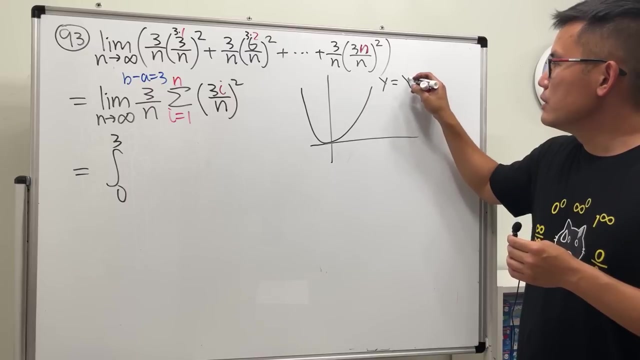 and uh, i'm going to perhaps just erase this and i'm going to just give you guys a picture right here real quick. so you see, when we have uh x to the some power, but it's actually just x plus third power. but no, no, no, no kidding just. 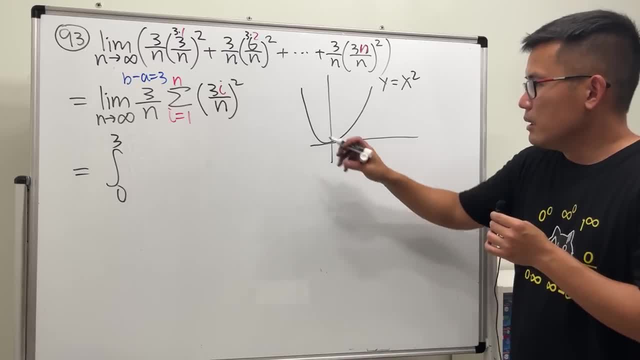 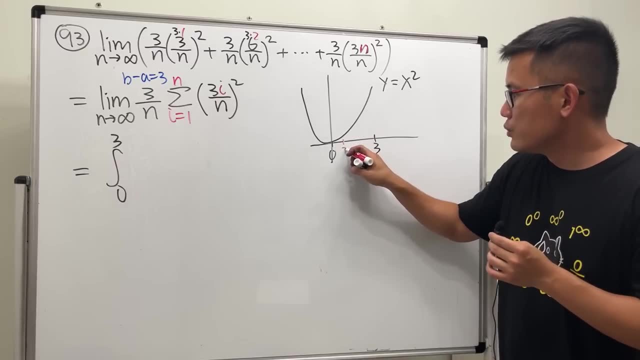 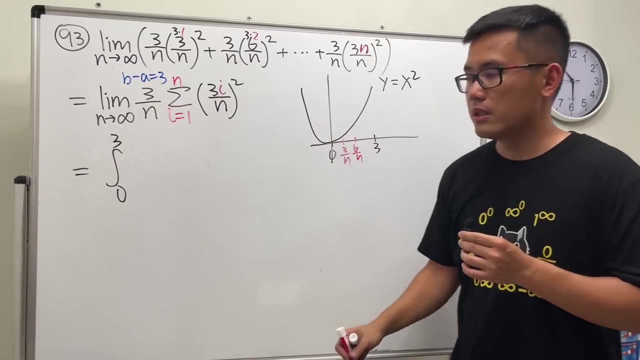 kidding. x to the second power, because we're going from zero to three, right, so each width is three over n, the next one is six over n. so you see, that's why i said, students, we match. so you see, you put this to the x value, we get that for. 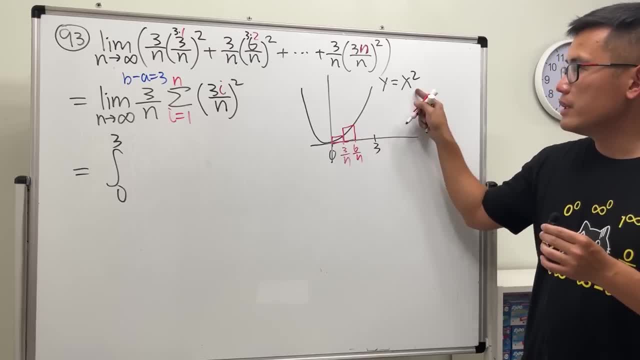 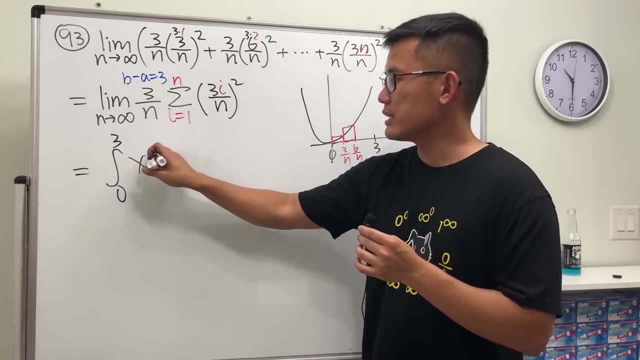 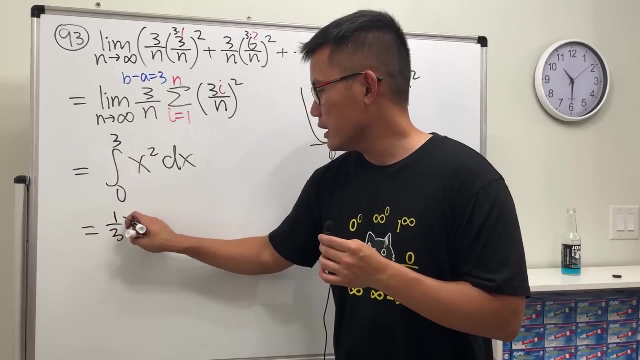 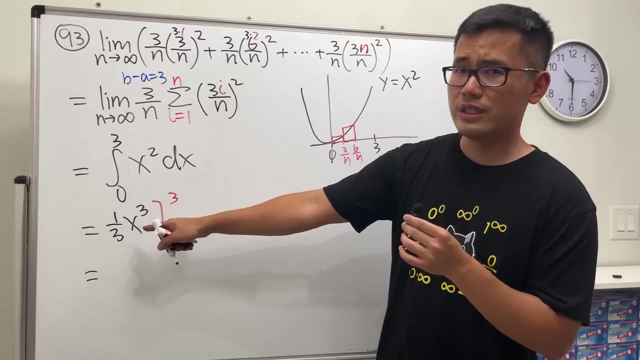 the height. you put this to be the x value. in here you get a height. so the function is actually just x squared. it's not three x squared. be really careful. so it's x squared, dx. work that out. one third x to the third power. zero to three plus three in here, three to the third power is 27. 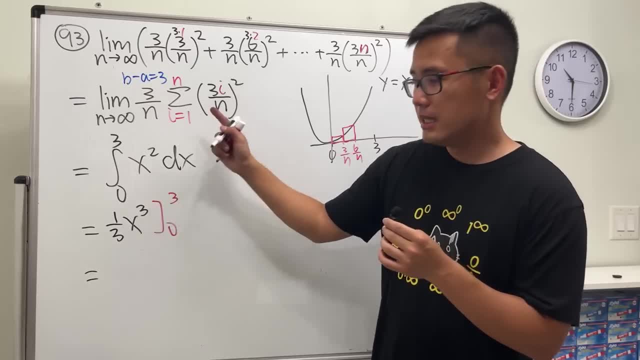 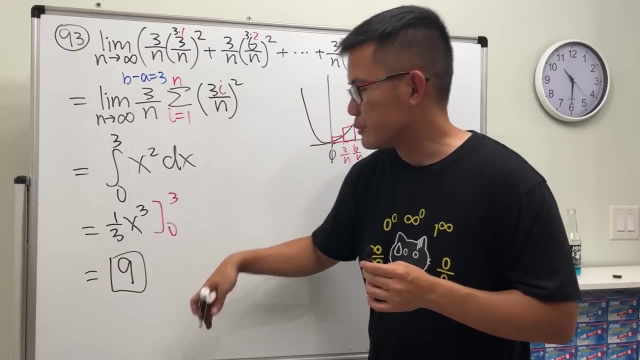 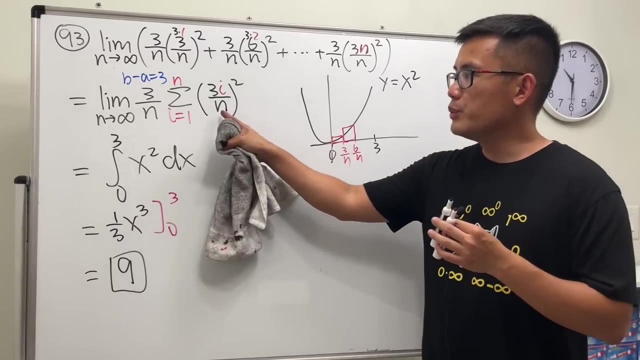 plus 3 in here, 3 to the third power is 27, divided by 3 is 9, and then subtract plug-in: 0, just 0. so yeah, we're good, we're good. so that's number 20, that's number 19: 3, so be really careful, huh, this and that match. what if we don't? 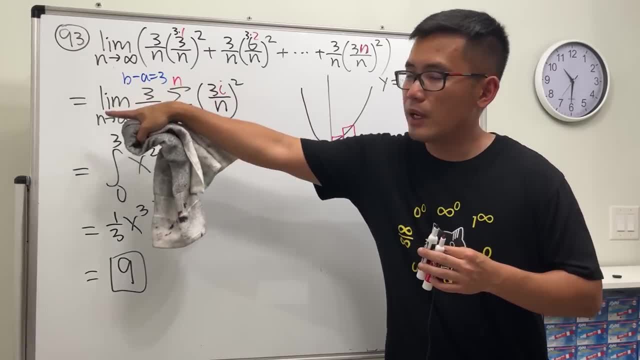 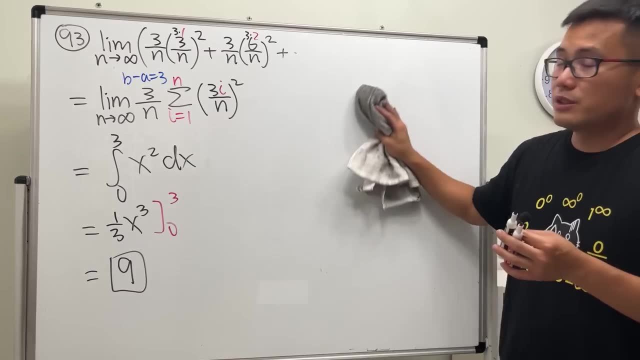 have a 3 right here. well, you can put this 3 on the very outside. that's that works too. but the reason that I have this 3 questions so similar is just because I want to go over this more details with you guys, so that way you 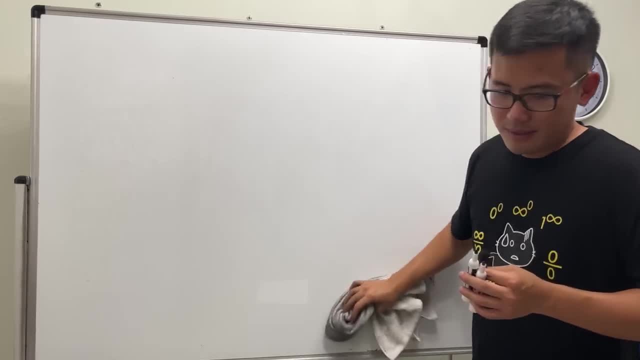 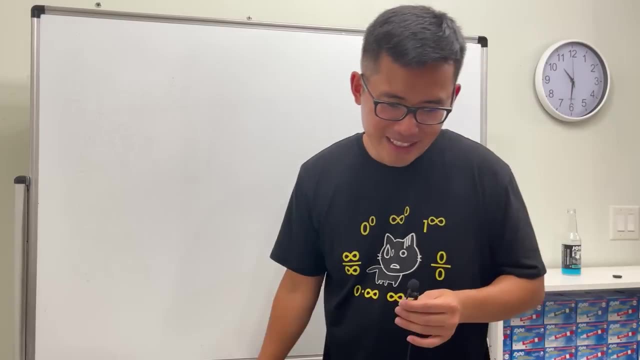 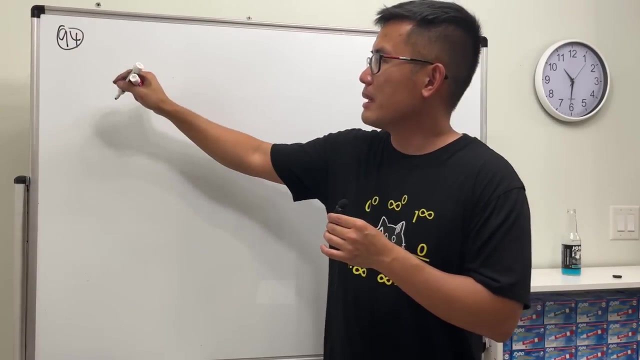 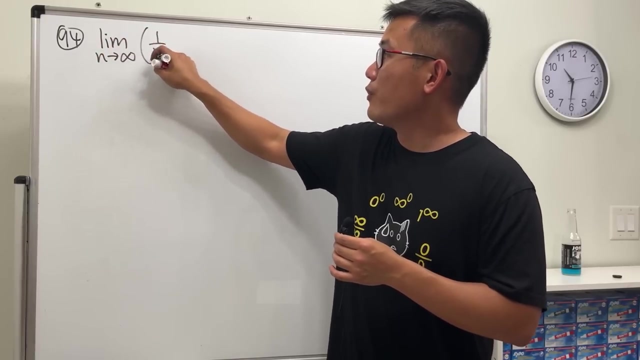 guys can fully understand what's going on. maybe you can see it here. I just have hurt my stomach already. I'm so hungry, okay. next I'm going to illustrate what I mean by if the numbers they don't match anyway. number 94: here we have limit and goes to infinity, 1 over. it's meant to be a 1, okay, oh the. 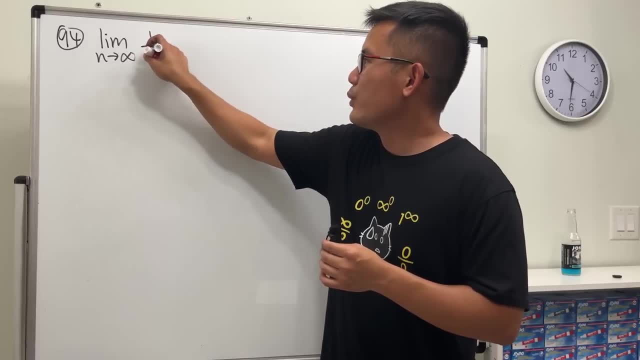 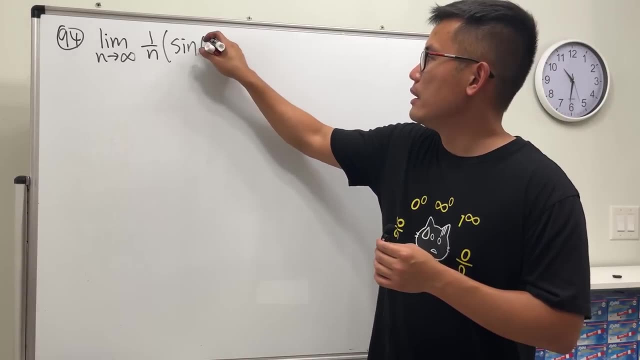 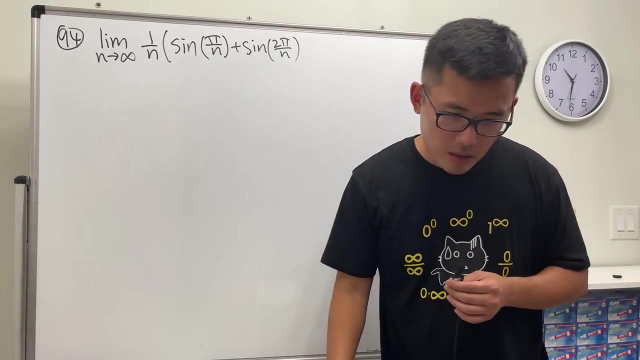 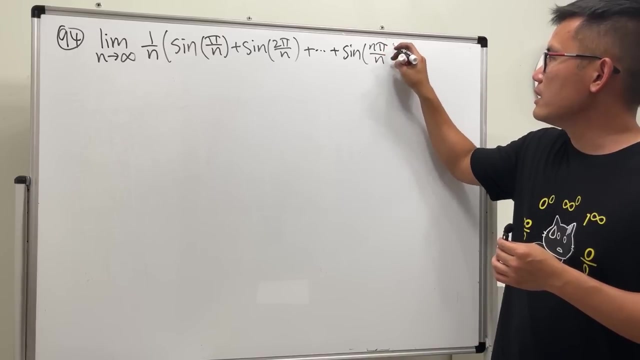 way I wrote it is this: I don't know why I wrote it as 1 over n, and then here we have sine pi over n, plus sine of 2 pi over n, and then sine of 3 pi over n, and then so on, so on, and then sine of n- pi. all right, let's put this in the sigma. 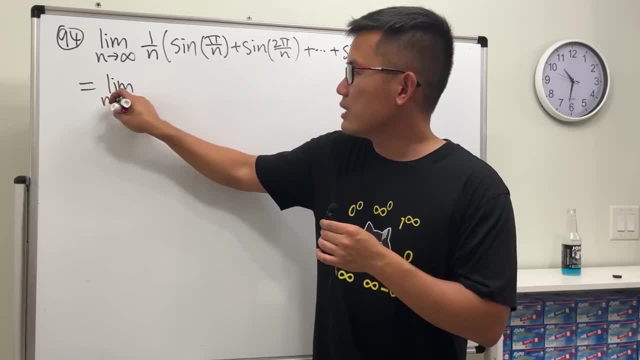 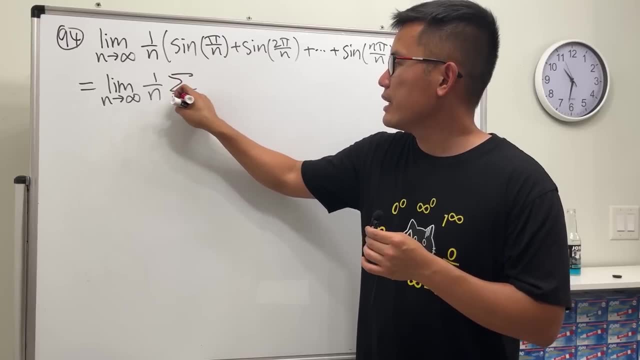 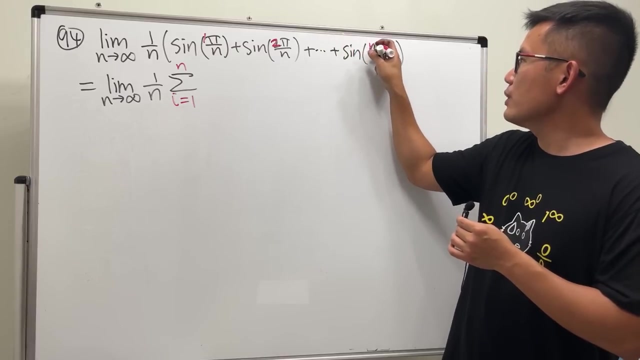 summation first, which is just the limit, as n goes to infinity, 1 over n, all this can be put it as the summation. i goes from 1 to n, 1 pi, 2 pi, 3 pi, so on, so on, so on, up to n pi. so we. 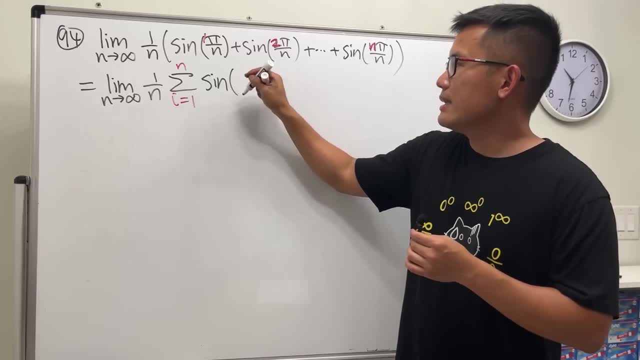 are talking about the sine of. let's put it as i PIł pi, i pi over n. now this number is gonna give us 1 nads, and as we have shown you that every size of p speaks the same, so weavez my solution: or zero, sorry, zero, plus richtige zum. 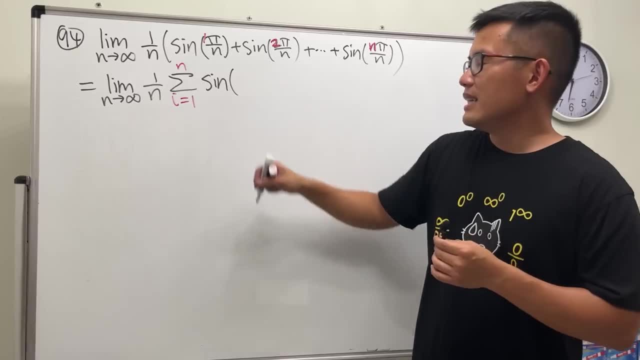 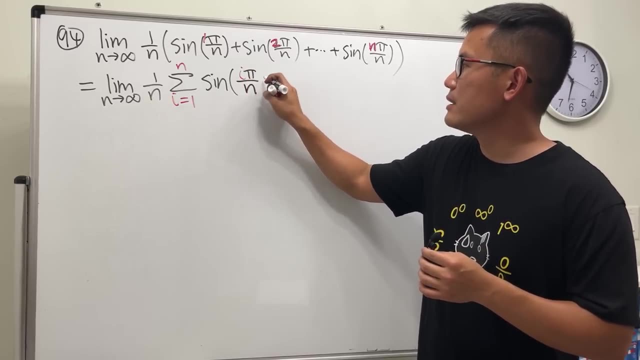 plus mit σ goes to 1 and phi goes to n, x is equal to zero. so this is sin of the force by 1 is equal to和, which is the Ih, and so on, and there areagan undaing that. but Iция is equal to H, sulla compatible to both, and sin of qa and at the endını healthy sum. so ей is equal to Psi and advert 167q, and I're done with the whole number. next we are talking about sine of. let's put this: i cards on the добрat. 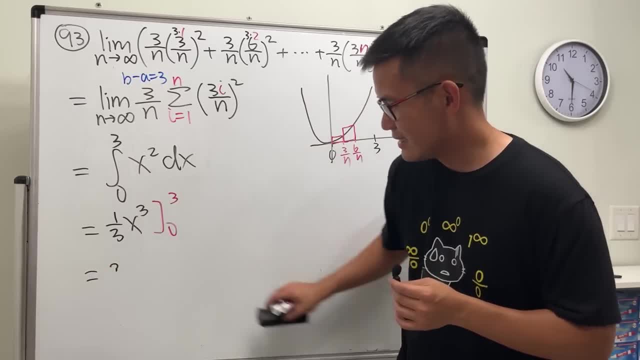 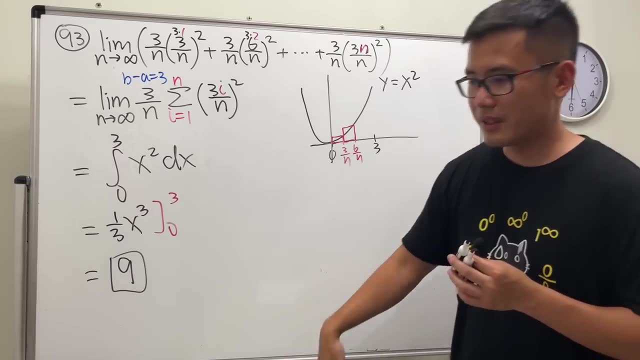 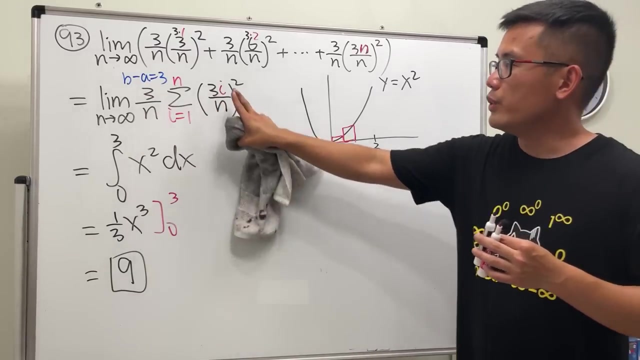 divided by three is nine, and then subtract, plug-in zero, just zero. so yeah, we're good, we're good. so that's number 20, that's number 19: three. so be really careful. huh, this and that match what? if we don't have a three right here, well, you can put this three on the very outside. that's that works too, but 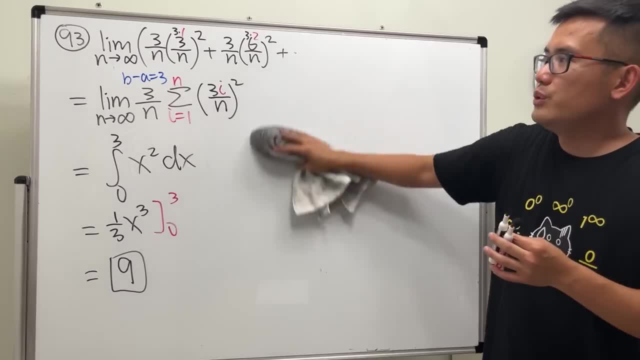 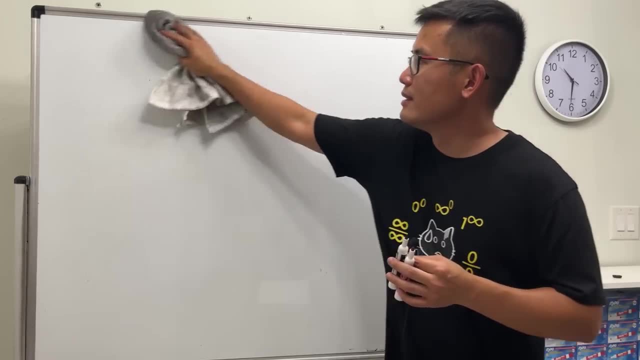 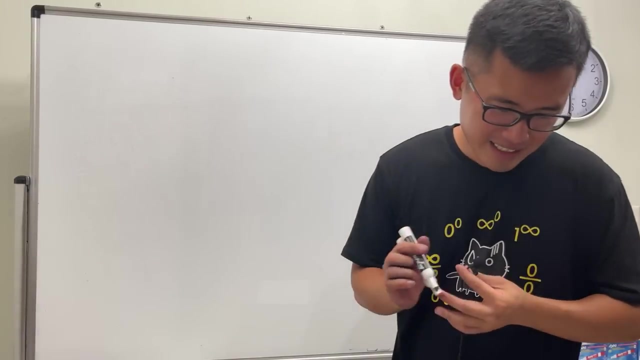 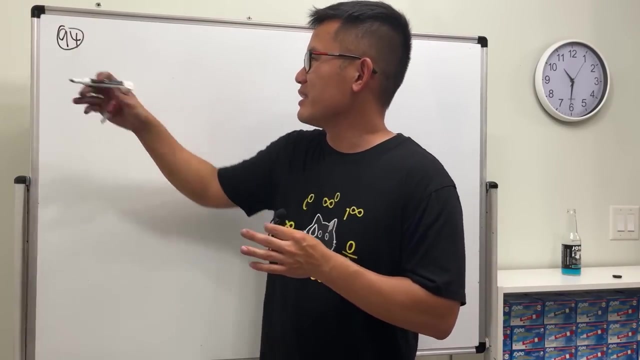 the reason that i have these three questions so similar is just because i want to go over these small details with you guys so that way you guys can fully understand what's going on. and maybe you guys have heard my stomach already. i'm so hungry anyway. next i'm going to illustrate what i mean by if the numbers they don't match anyway. number 94: 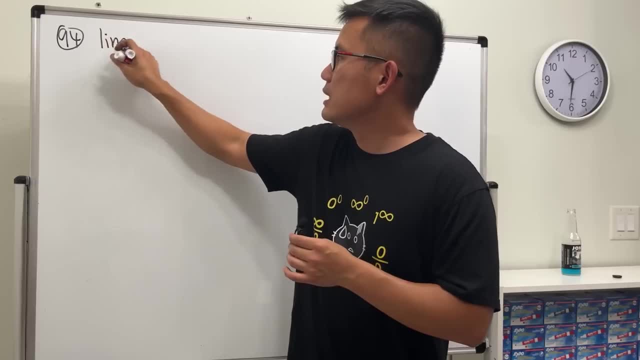 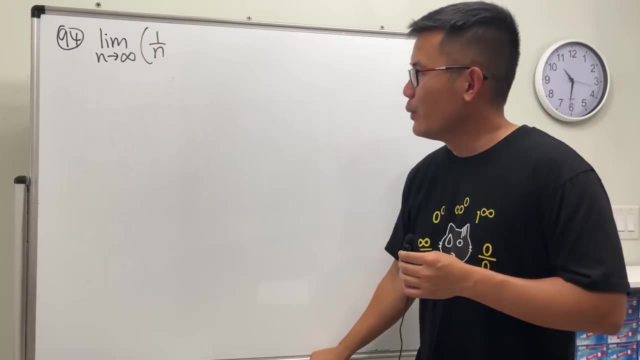 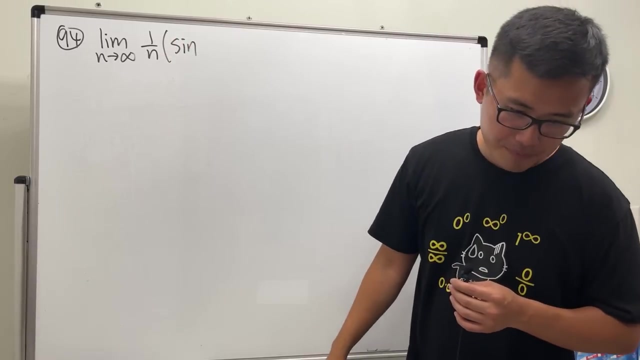 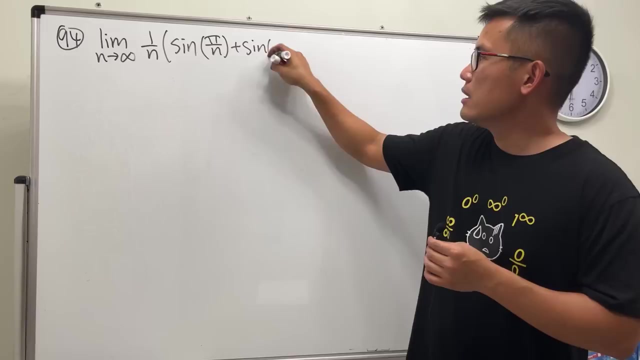 here we have limit and goes to infinity, one over. it's meant to be a one. okay, oh, the way i wrote it is this. i don't know why i wrote it as one over n. and then here we have sine pi over n, plus sine of two pi over n, and then sine of three pi over n. 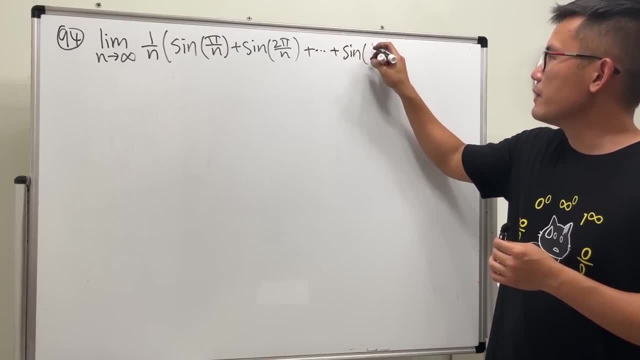 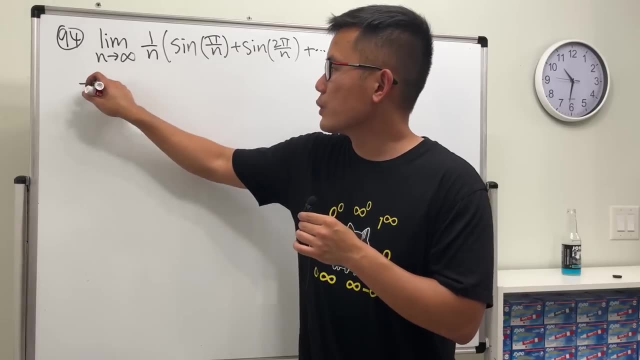 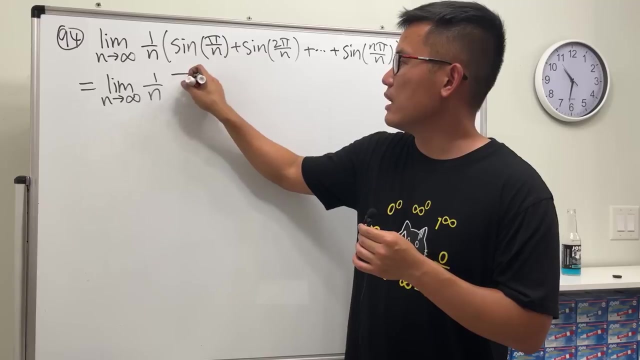 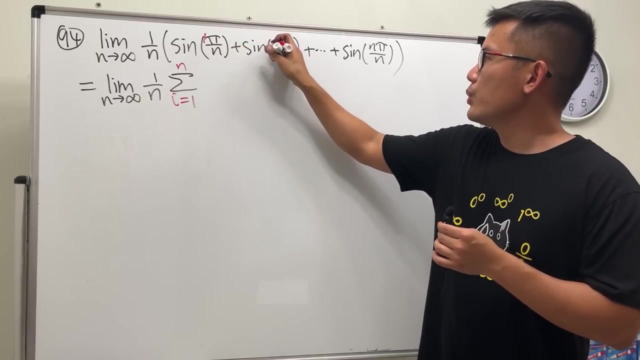 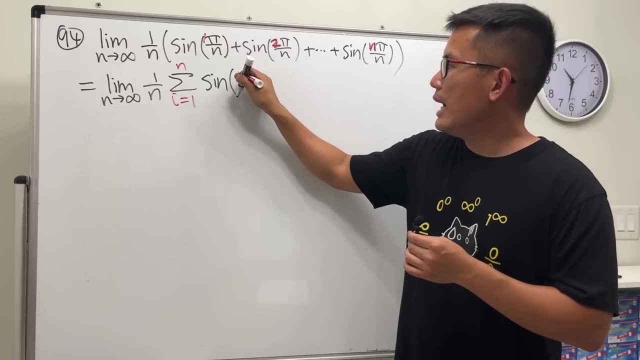 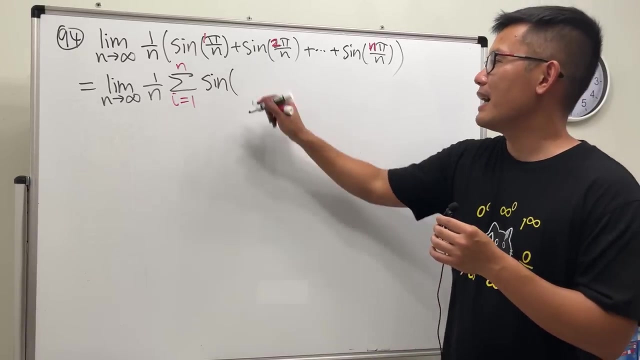 and then so on, so on, so on, and then sine of n pi. all right, let's put this in the sigma: one summation first, which is just the limit, as n goes to infinity, 1 over n. All this can be put it as the summation. i goes from 1 to n, 1 pi, 2 pi, 3 pi, so on, so on, so on, up to n pi. So we are talking about sine of. let's put it as i pi or pi i. i pi over n. 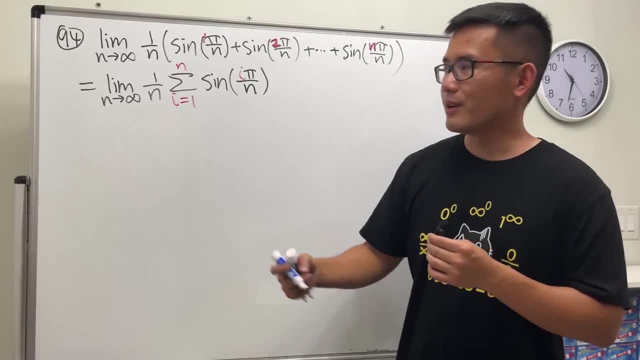 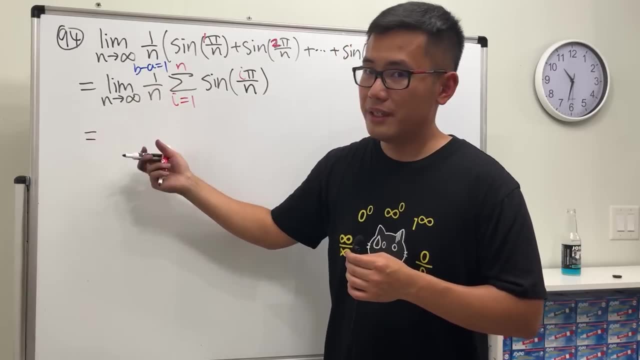 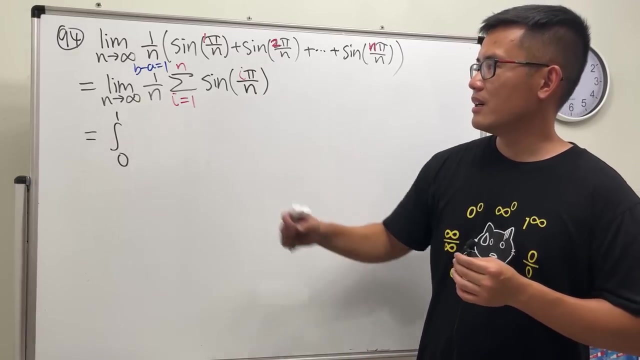 Now this number is just 1, and that so means b minus a is equal to 1.. So this right here is equal to what Integral going from 0 to 1 only? Now the hard part is: what's the function? Is it sine of x or sine of pi x? 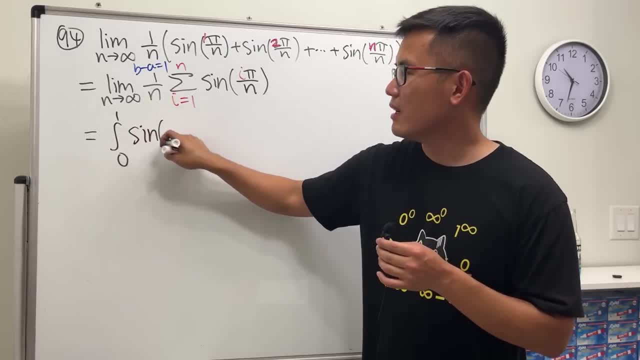 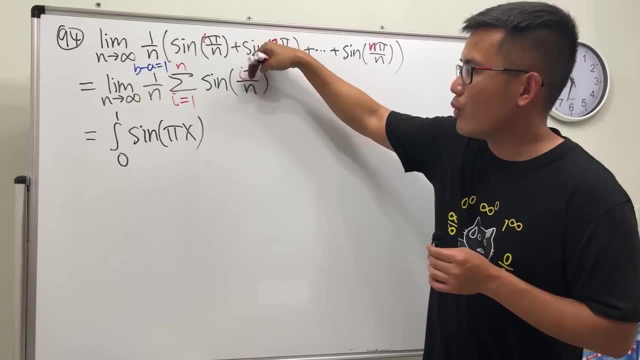 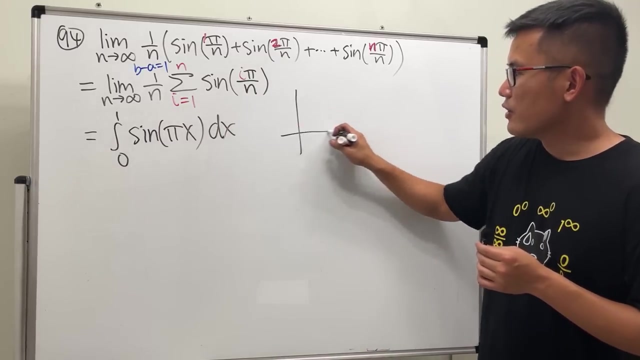 The answer is: sine of pi x. If this is a 1, this pi will just be the coefficient. and look at the i over n, which is that will give you the x. I'll convince you guys that this is actually legit Sine of pi over x. let's just say it looks like this, somewhat like that. 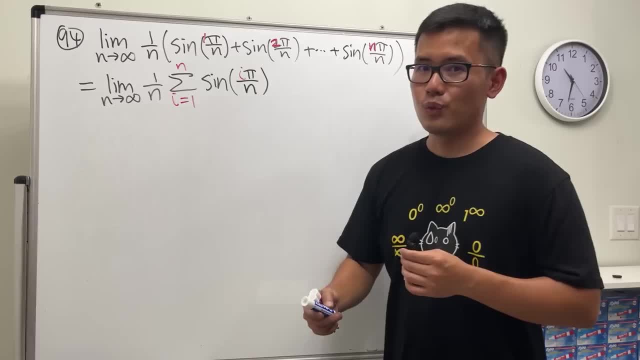 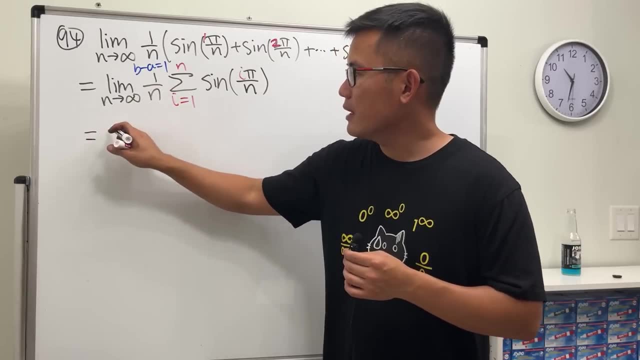 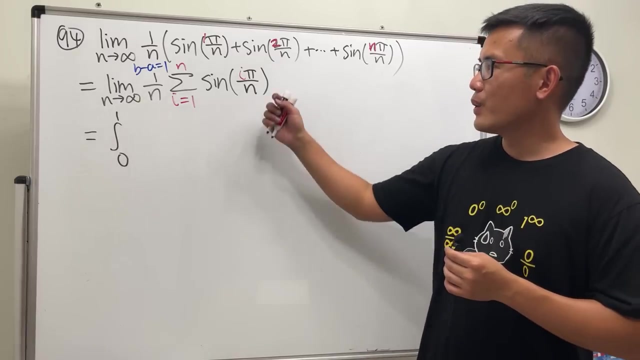 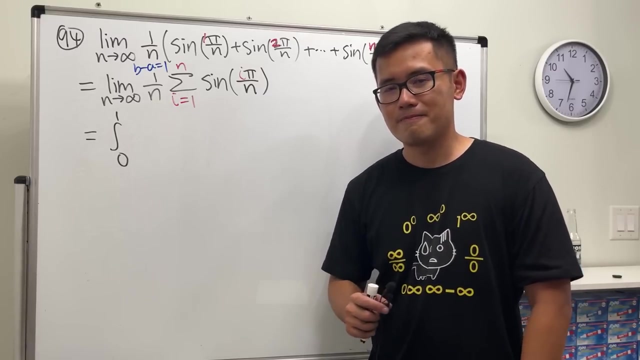 now this number is just one, that's all means. b minus a is equal to one. so this right here is equal to what integral going from 0 to 1? only now the hard part is: what's the function? this is sine of X or sine of pi X. the answer is sine of. 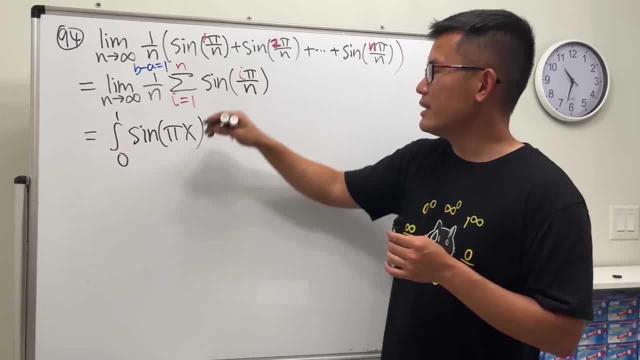 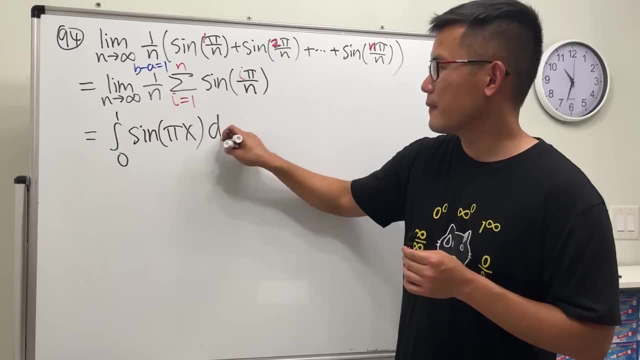 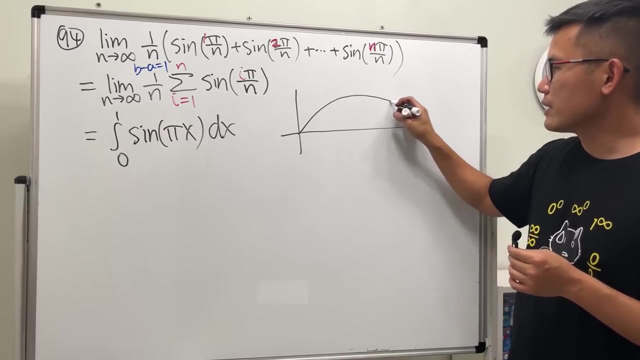 pi X. if this is a 1, this pi will just be the coefficient. and look at that: I over n, which is: don't give you the X, I'll convince. guess that this actually the jet sign of pi over X. let's just say it looks like this, somewhat like that: 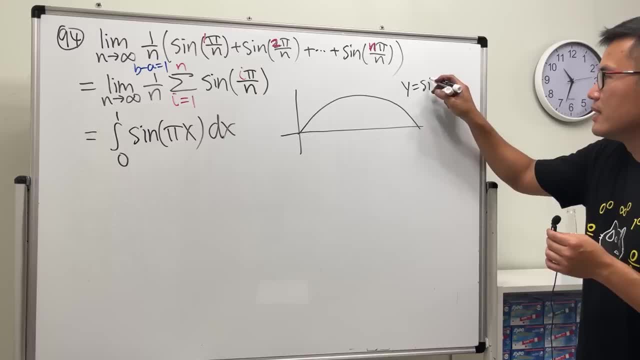 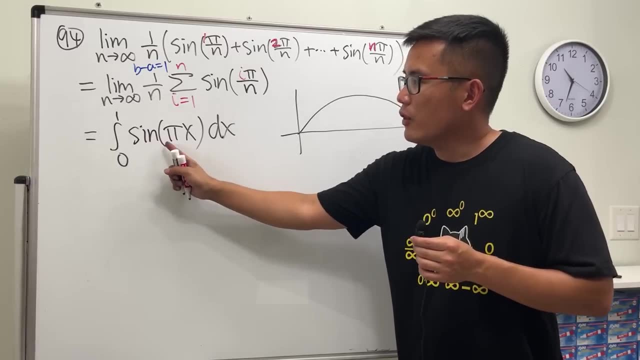 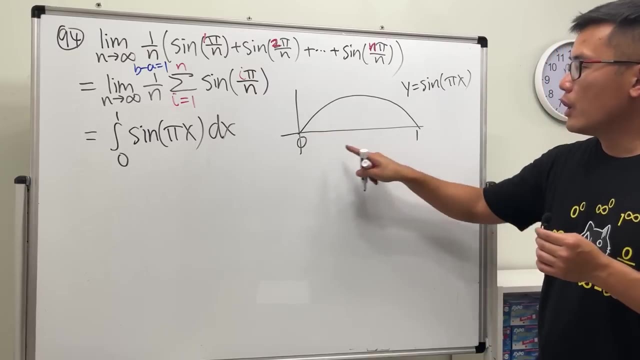 hopefully this is the jet. if not, I will have to correct it. I'm tired, so we'll see. so you see, we have sine of pi over, we have sine of pi X. so this is the curve and the deal is that we are going from 0 to 1. when X is 1, sine of pi is 0. so we do have this. 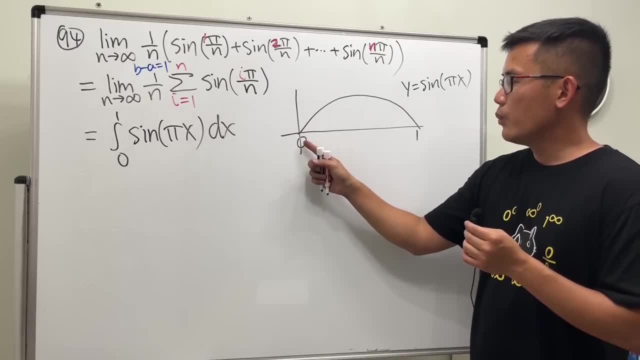 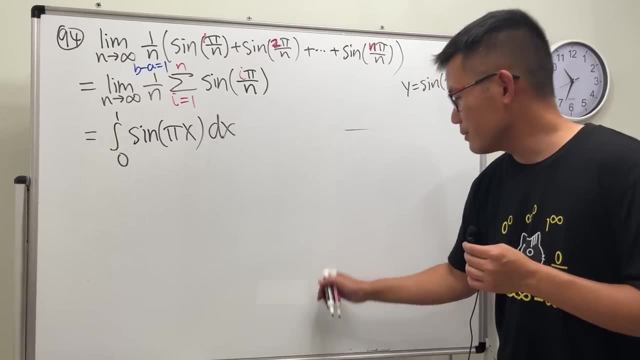 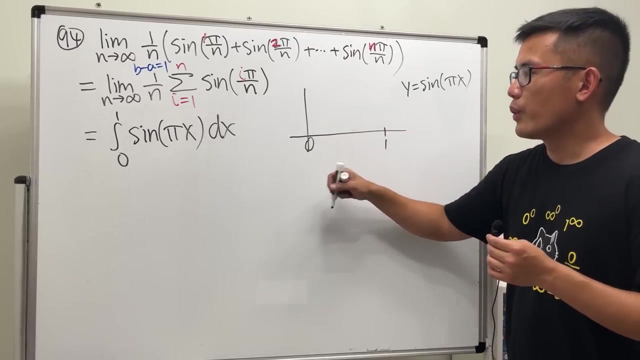 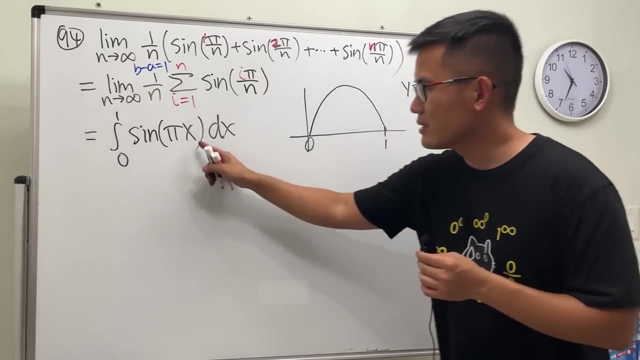 part right here. okay, we want to have. oh, the picture is wrong. yeah, let me. let me try to try study more realistic. because this is 0, I say this is 1, and when X is 1 over 2, you get one sort. when X is 1 over 2, you get sine of pi over 2, which is the 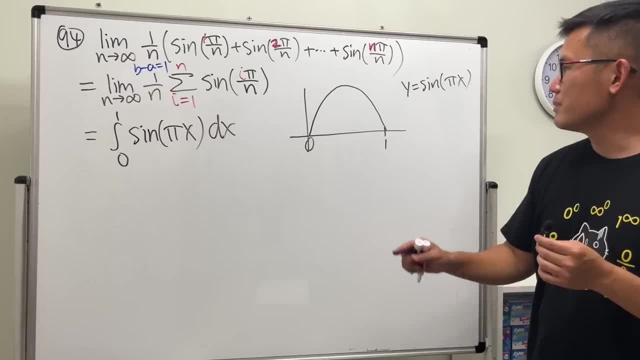 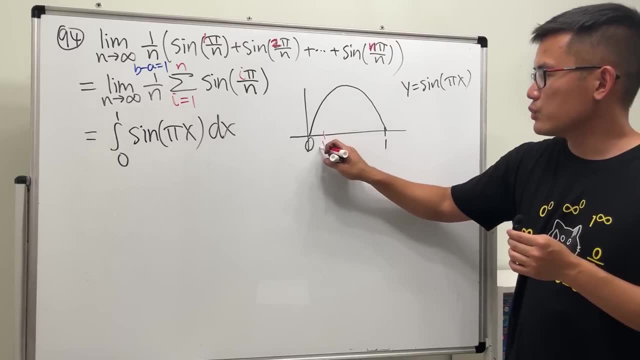 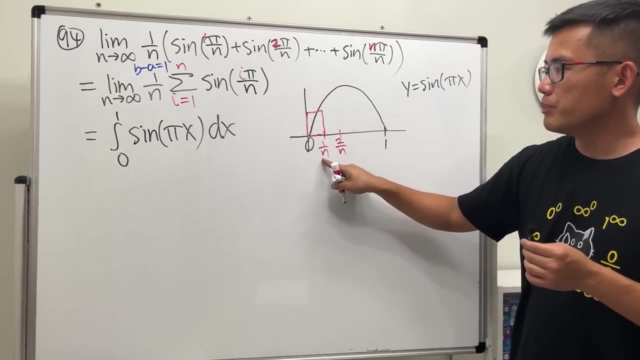 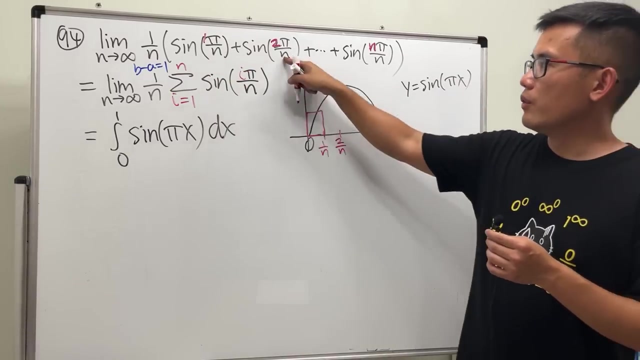 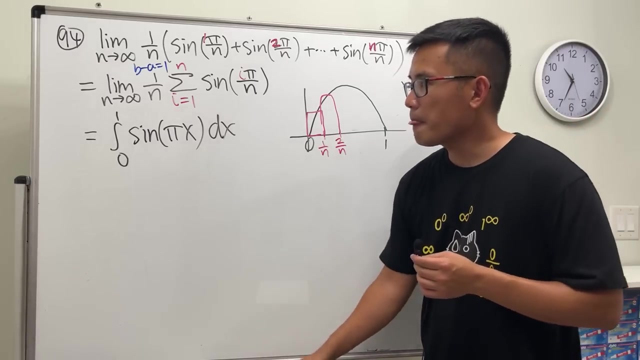 one doesn't matter, trust the computation, other stuff. anyway, going for travel to 1, this right here is one over and two of n, thank you, and and so on. put this into this X pi over, and put us into here 2 pi over n, and so on, so on, so on, okay, okay, yeah. so i want to see how many of you guys are still. 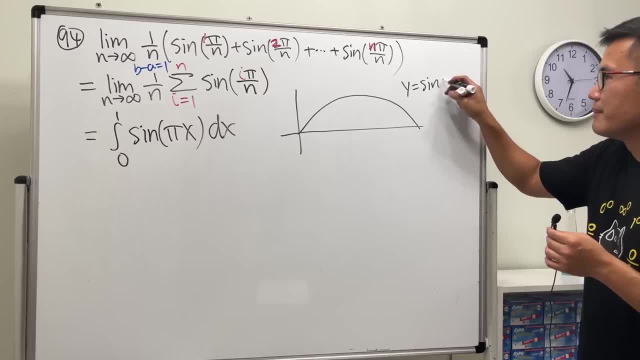 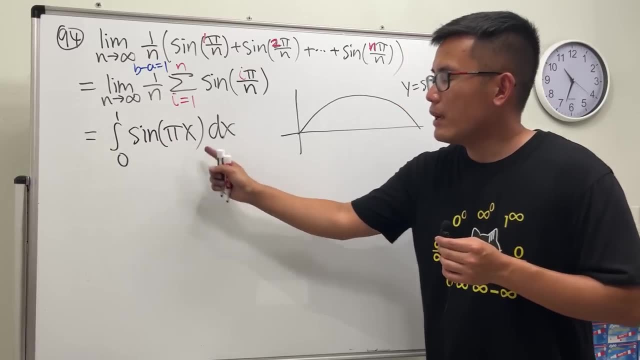 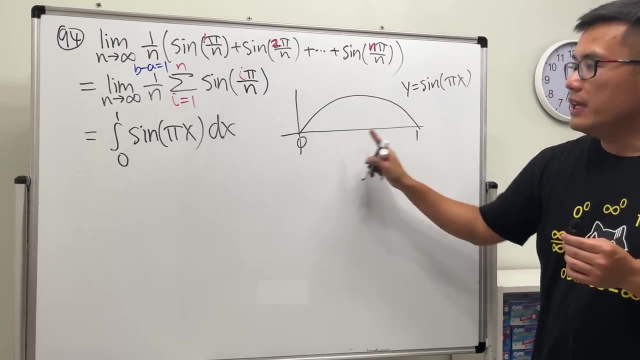 Hopefully this is legit. if not, I will have to correct it. I'm tired, so we'll see. So you see, we have sine of pi. so this is the curve, and the deal is that we are going from 0 to 1.. When x is 1, sine of pi is 0, so we do have this part right here. 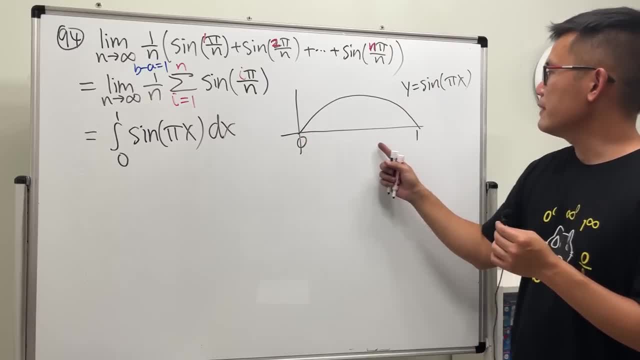 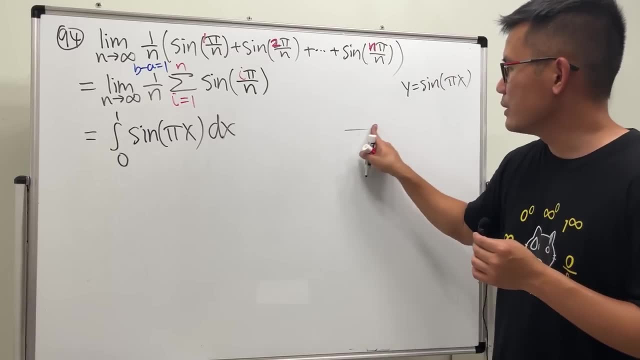 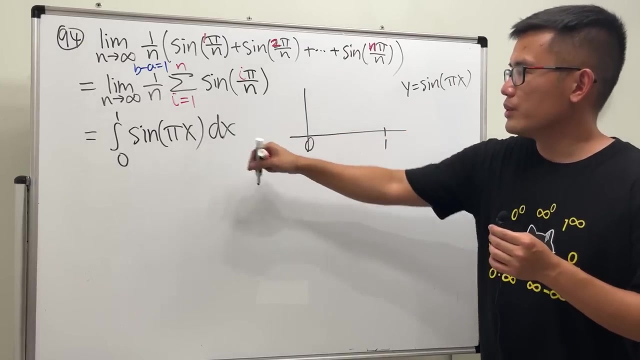 Okay, we want to have. oh, the picture is wrong. Let me try to draw it slightly more realistic. because this is 0,, let's say this is 1, and when x is 1 over 2, you get 1,, so this is 1.. 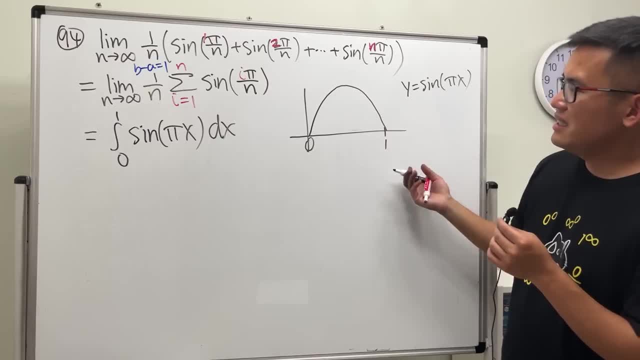 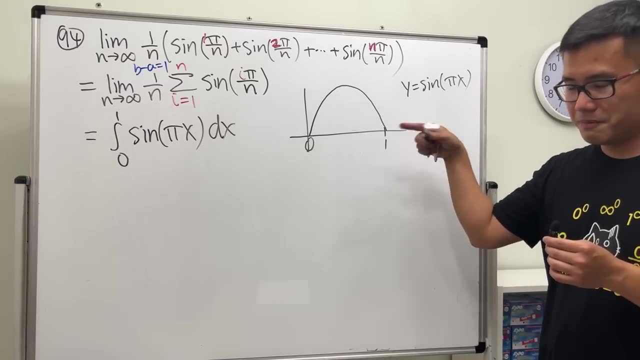 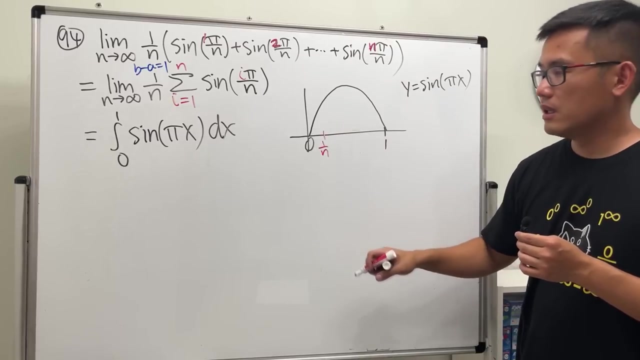 So when x is 1 over 2, you get sine of pi over 2, which is 1.. Doesn't matter, trust the computation and all that stuff. Anyway, going from 0 to 1, this right here is 1 over n, 2 over n, 0 over n, and so on. 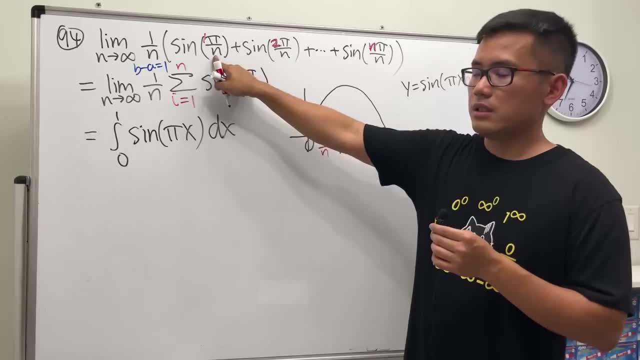 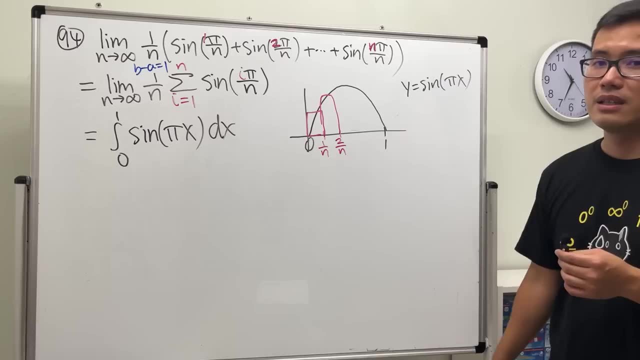 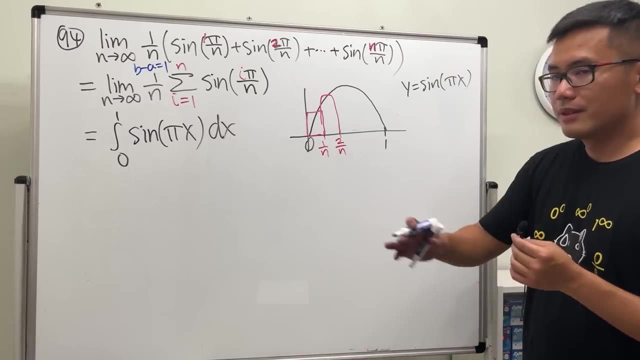 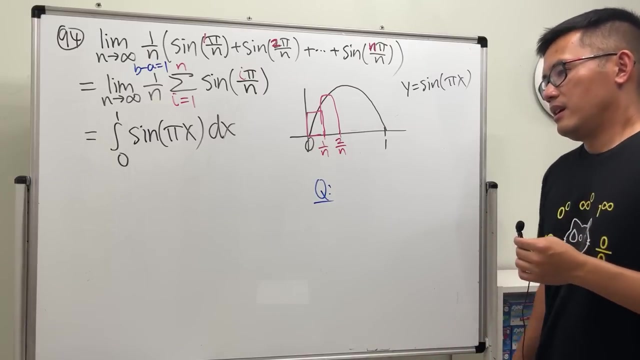 Put this into this: x pi over n. Put this into here: 2 pi over n, And so on, so on, so on. Okay, Okay, Yeah. So I want to see how many of you guys are still- uh, I want to see how many of you guys are still watching this. 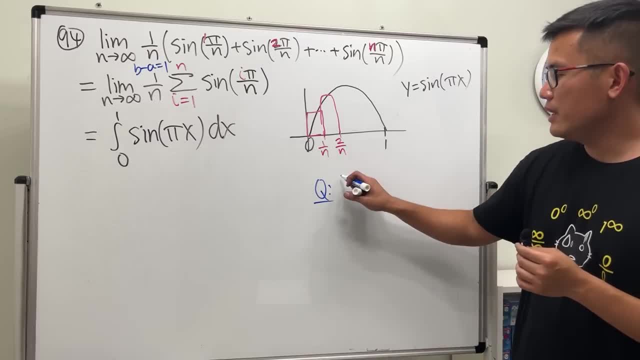 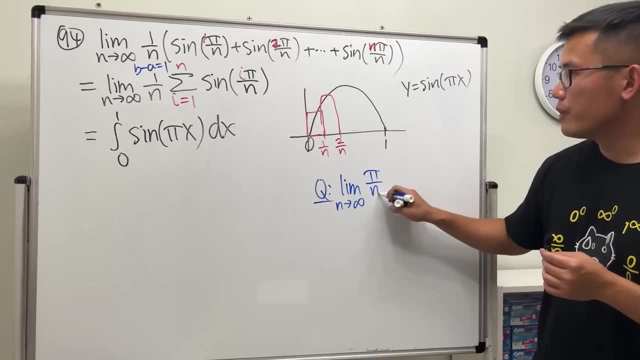 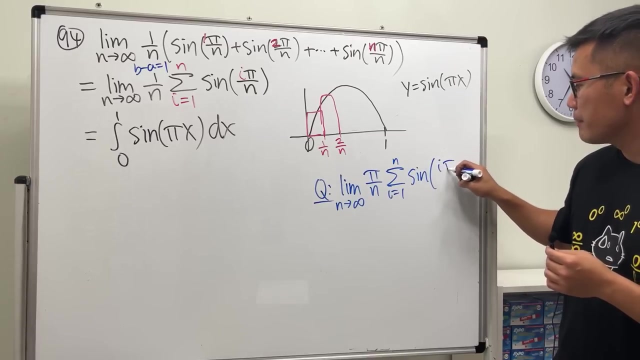 Question for you guys. What if today we have the limit as n goes to infinity? What if we have a pi here and over n and the summation i goes from 1 to n and then, sine of i, pi over n. so tell me what the function is and tell me from where to where. 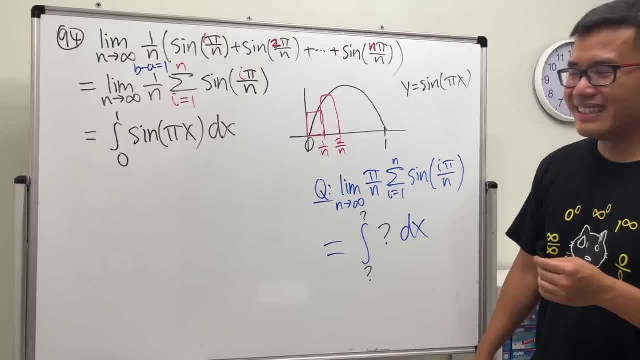 i'll give you guys the dx there. do not just put the pi at the front, just say, hey, that's the answer. multiply by pi. don't do that. don't do that. do the things i said that. it's better that way. so the range will be going from: 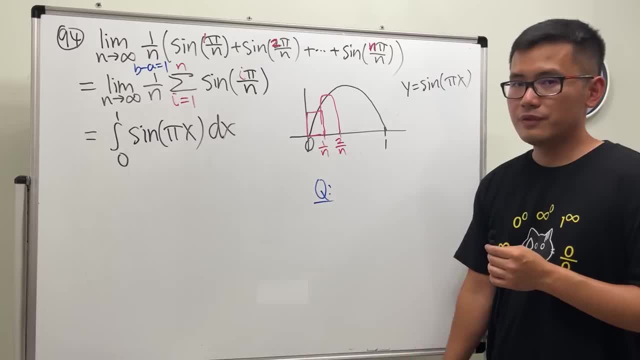 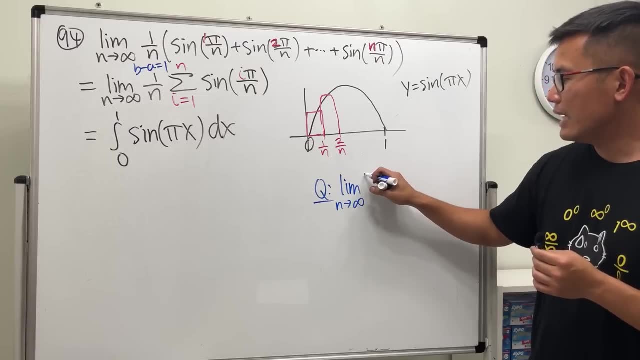 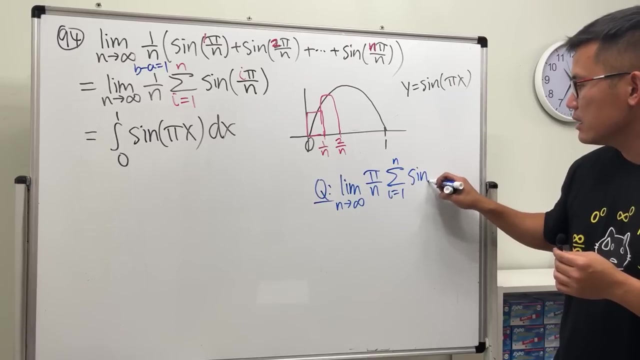 i want to see how many of you guys are still watching this question. for you guys, what if today we have the limit as n goes to infinity? what if we have a pi here and over n and the summation i goes from 1 to n and then sine of i pi over n. so tell me what the function is. 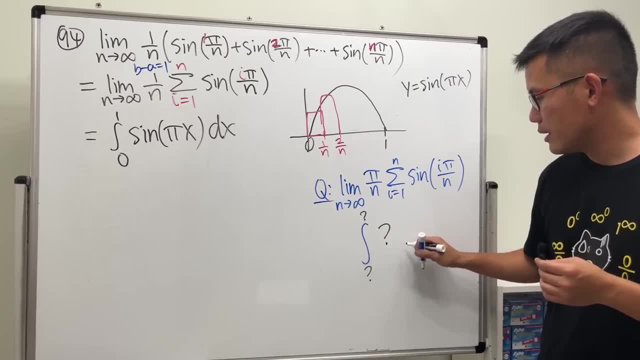 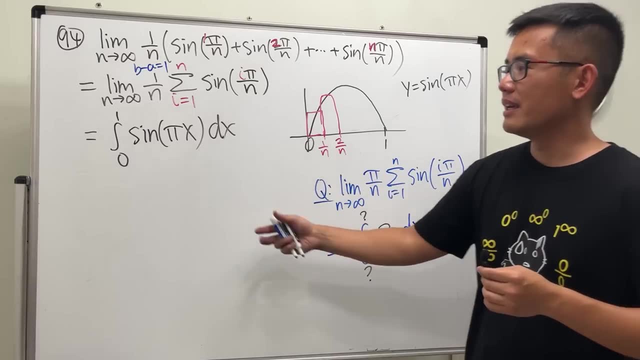 and tell me from where to where. i'll give you guys the dx there. do not just put pi at the front and just say, hey, that's the answer. multiple pi by pi. don't do that. don't do that. do the things i said that it's better that way. 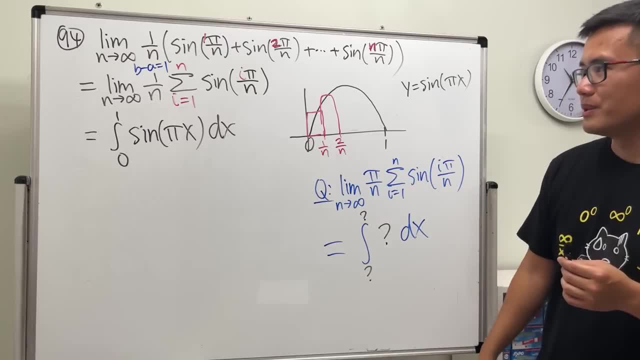 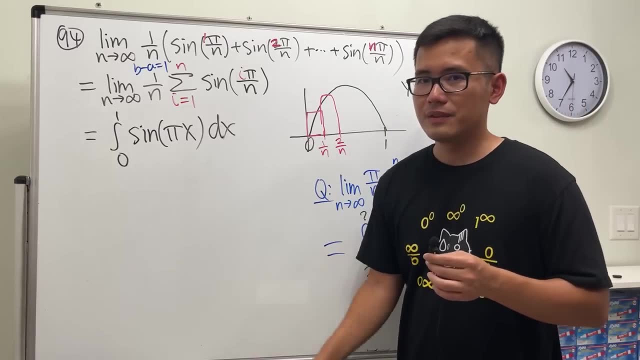 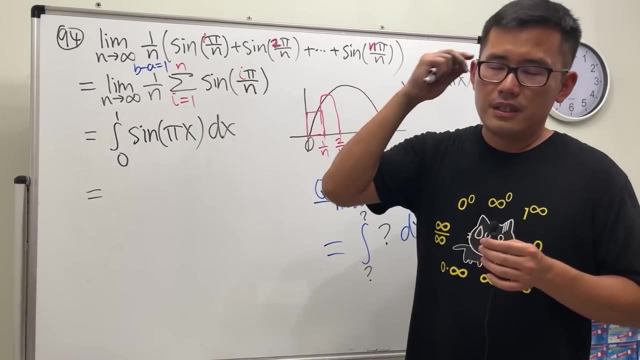 so the range will be going from 0 to pi. okay, the range will be going from 0 to pi, and tell me what the function is. but anyway, though, what's the answer for this? all right, i'll show you guys how to do this. anti-derivative of sine is negative cosine. 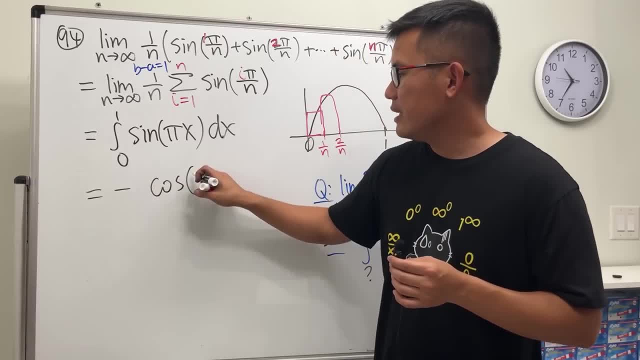 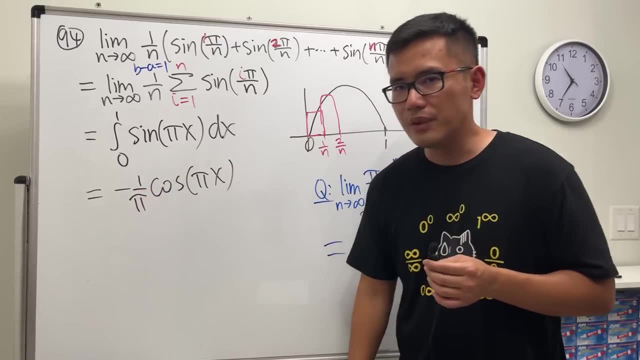 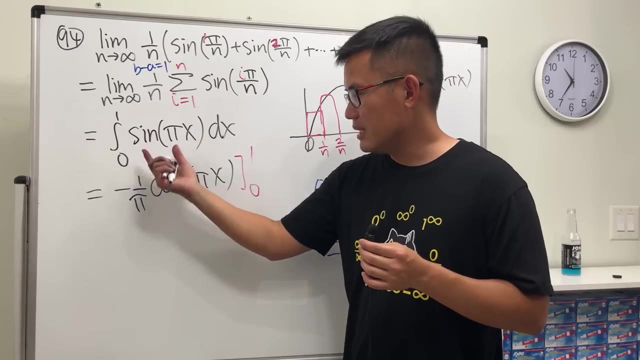 because the derivative negative cosine is positive sine and then the input is pi x. but we will have to divide by this constant here. how do we do all the entire derivative of that? i have 100 integrals already, by the way. trust me, this right here is the answer for that. 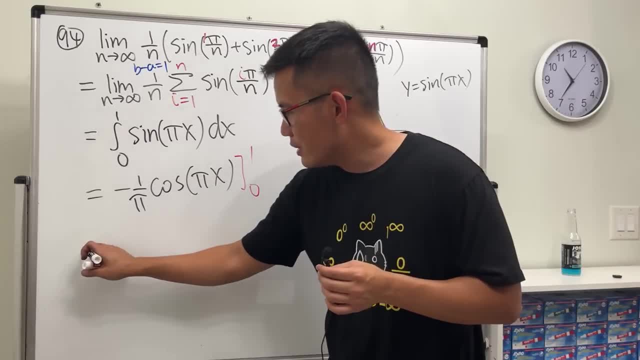 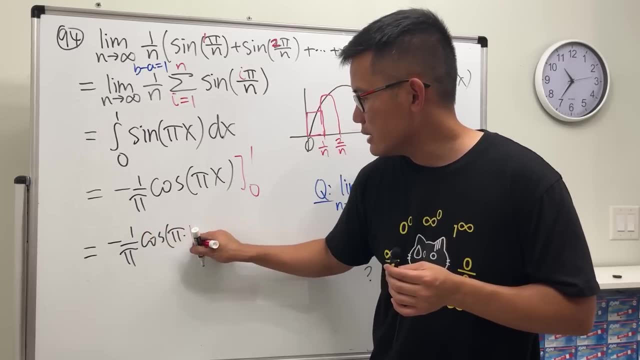 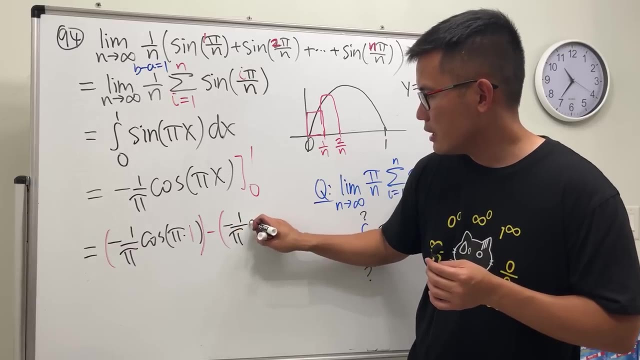 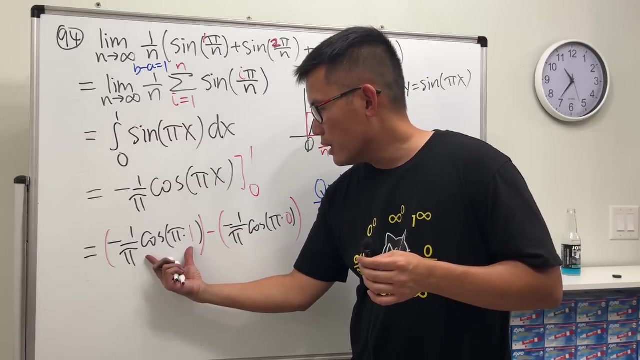 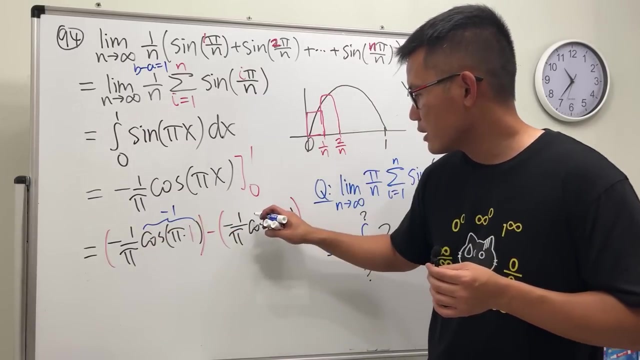 yes, now put the one, put the zero. so here be really careful though. one over negative, one over pi. cosine of pi times one. that's the first part minus. put a zero. so we have negative one over pi cosine of pi times zero. okay, cosine of pi is negative one. cosine of zero, pi times zero is zero is one. 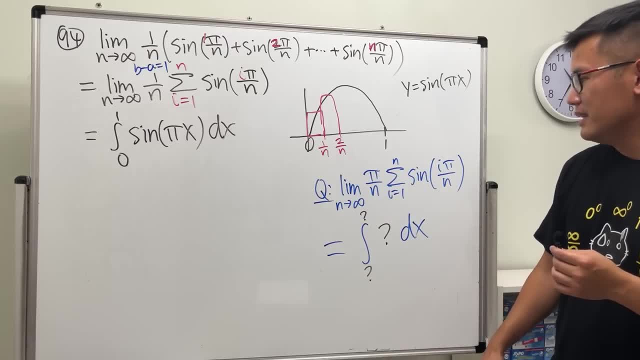 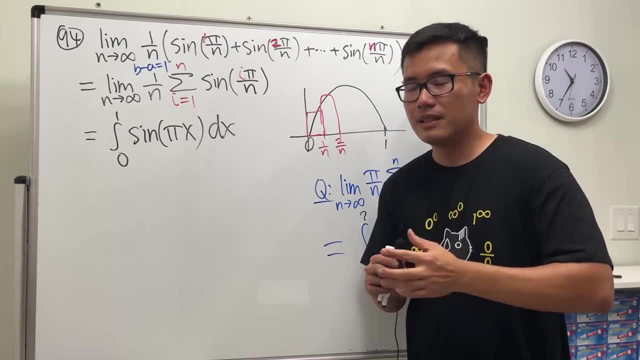 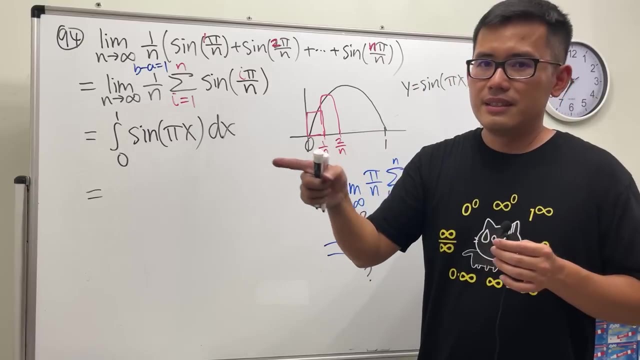 0 to pi. okay, the range will be going from 0 to pi, and then tell me what the function is. but anyway, though, what's the answer for this? all right, i'll show you guys how to do this. anti derivative of sine is negative cos, because the derivative negative cosines positive sine, and then the input is: 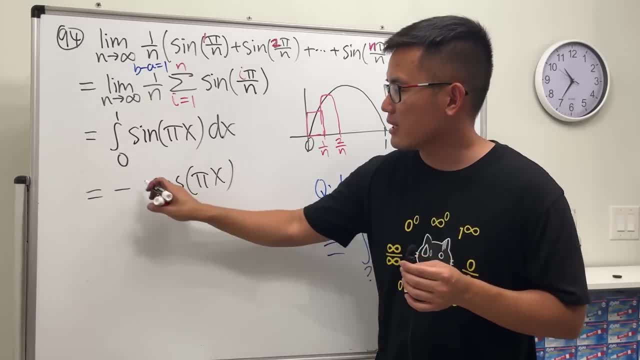 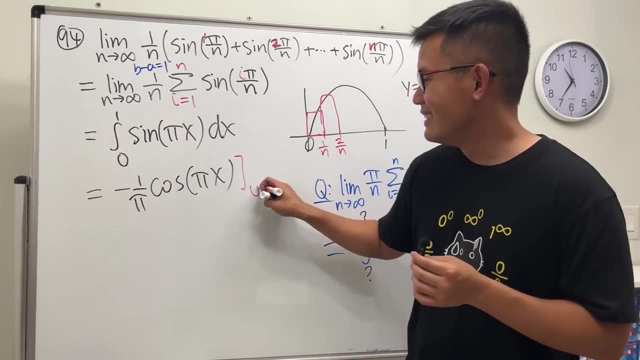 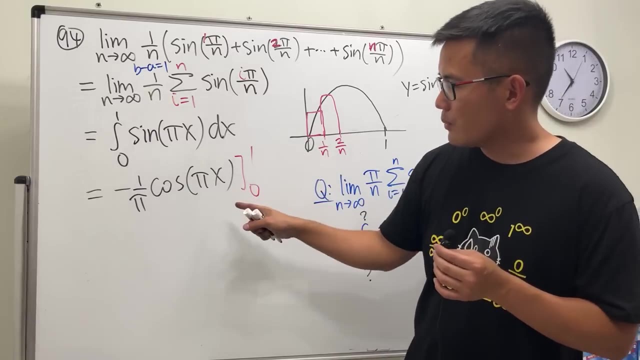 pi x, but we will have to divide by this constant here. how do we do all the entire derivative of that? i have 100 integrals already, by the way. trust me. this right here is the answer for that. yes, now put the one, put the zero. so here, be really careful though. 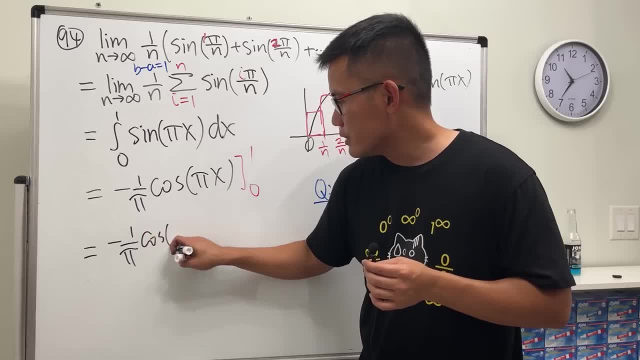 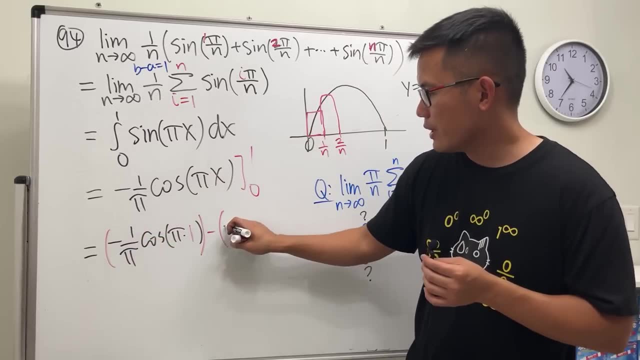 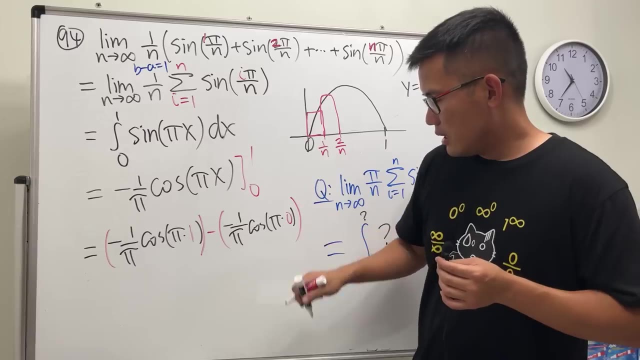 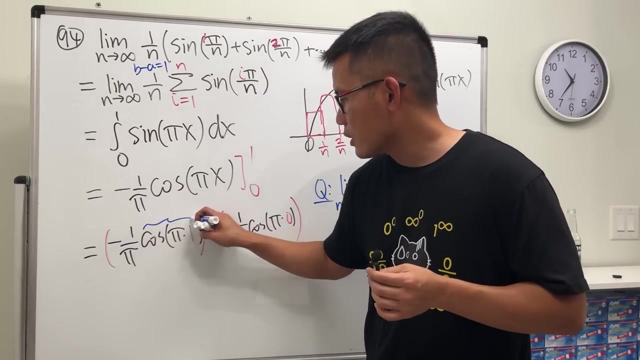 one over negative, one over pi. cosine of pi times one, that's the first part minus put a zero. so we have negative one over pi cosine of pi times zero. okay, cosine of pi is negative, one. cosine of zero, that's pi times zero, zero is one. so 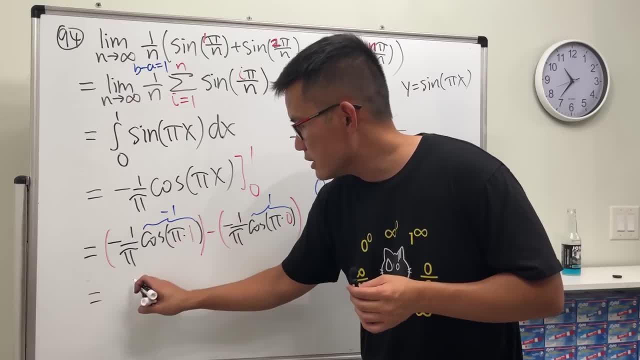 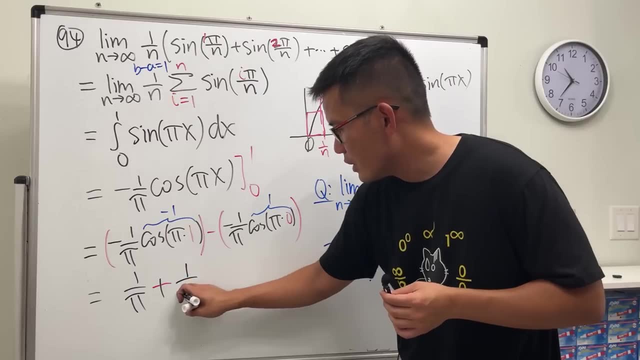 here this, right here, gives us positive one over pi. so here this right here, gives us positive one over pi. so here this, right here, gives us positive one over pi. and then negative, negative and then negative, negative and then negative. negative becomes a positive one over pi, becomes a positive one over pi. 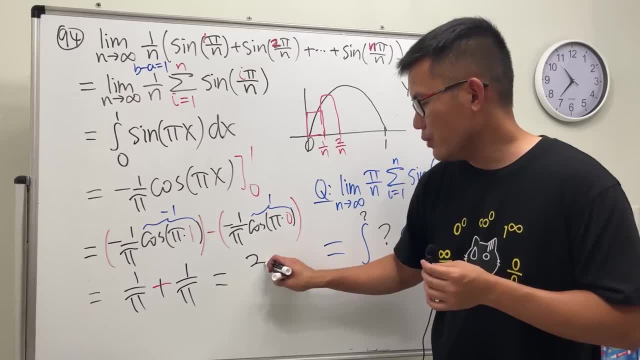 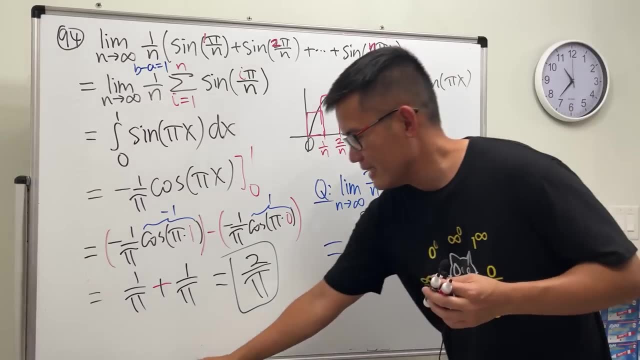 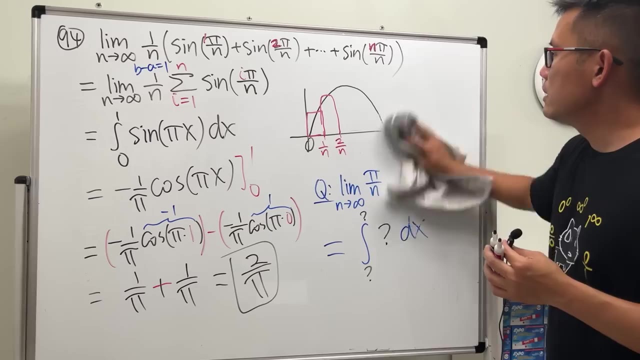 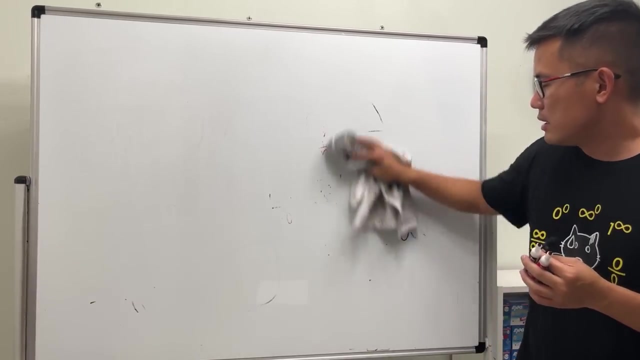 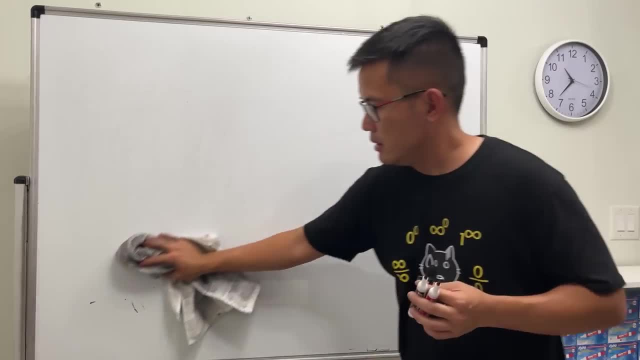 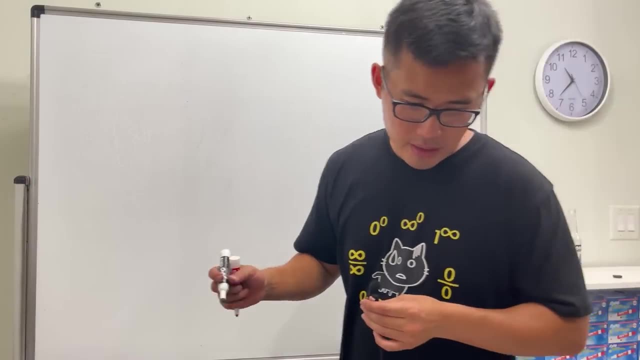 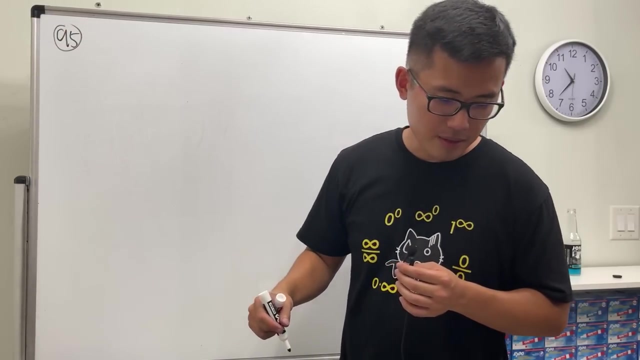 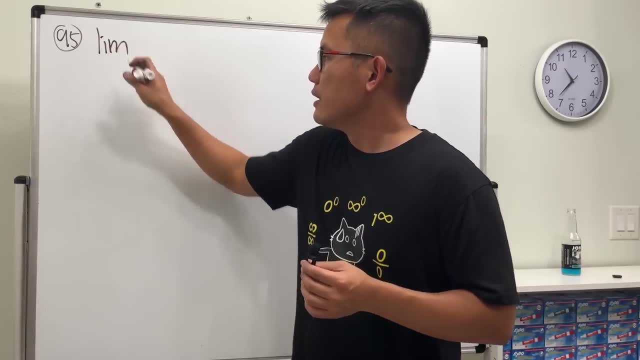 is uh better that way is uh better that way. so we have the limit, so we have the limit. so we have the limit. let me just see. i don't know why. i just let me just see. i don't know why. i just let me just see. i don't know why. i just want to check. wow, seven hours. 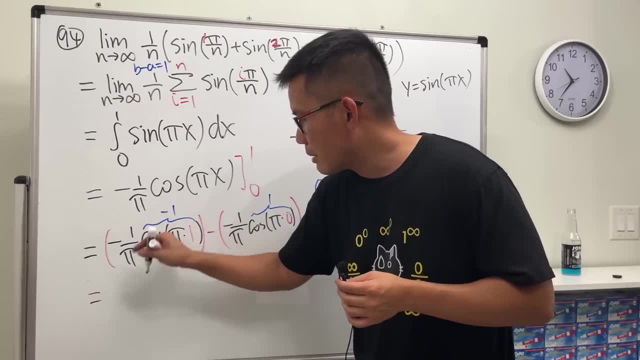 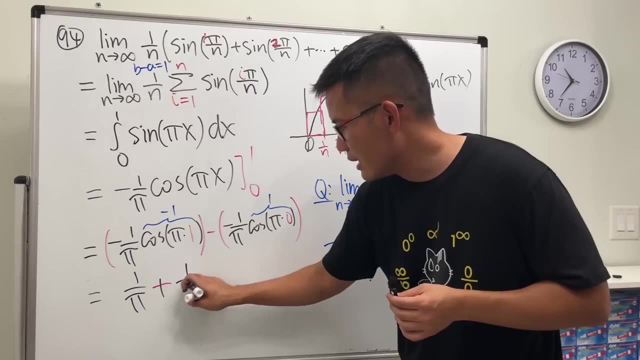 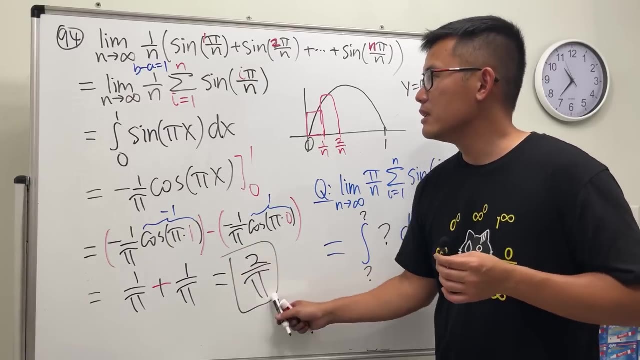 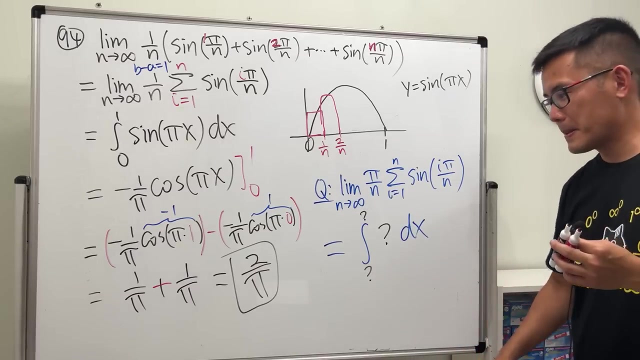 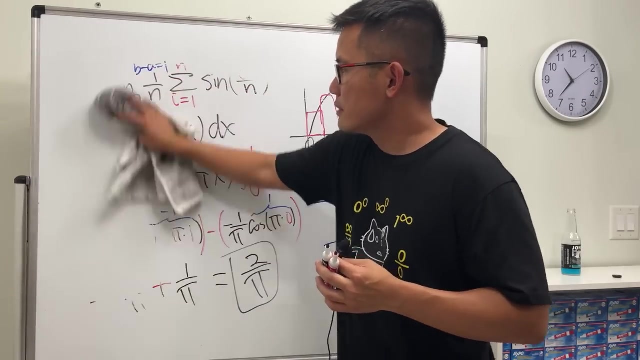 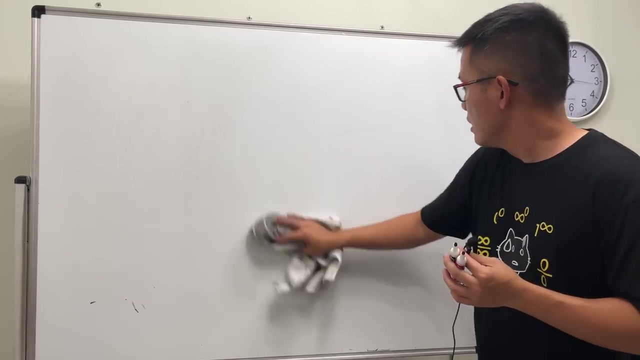 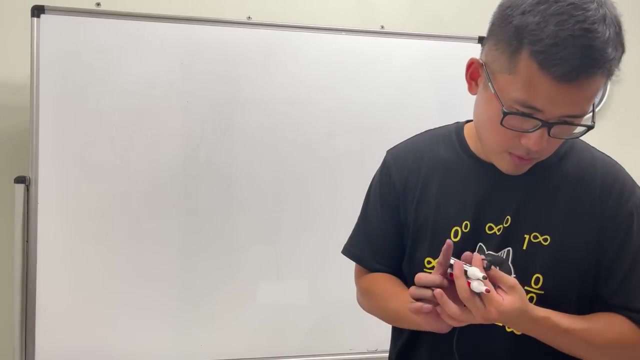 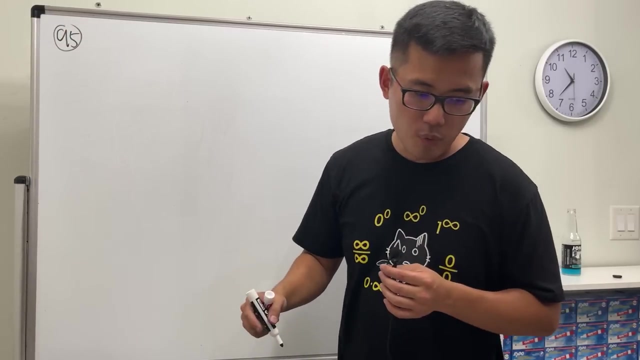 so here this right here gives us positive one over pi, And then negative, negative becomes a positive 1 over pi. Wow, this was crazy. The answer for that is 2 over pi. How pretty is this? Cool huh. All right now, I'm just going to put the question in the summation form. 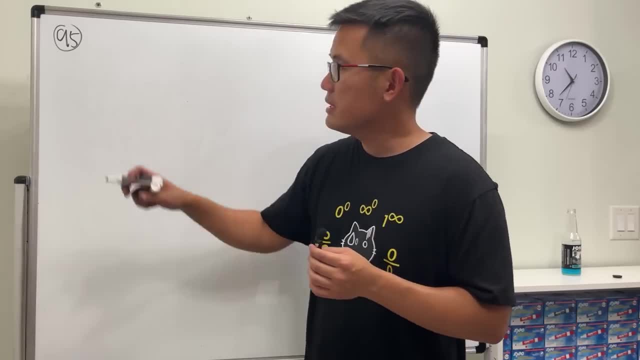 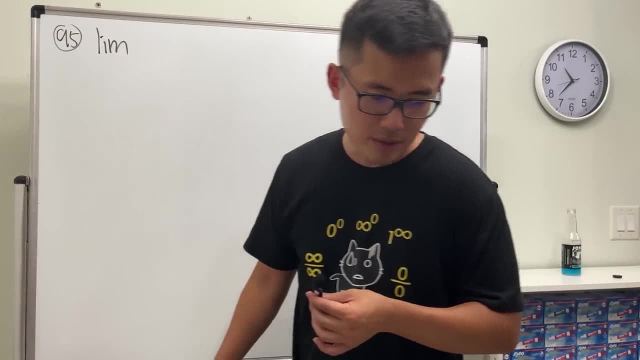 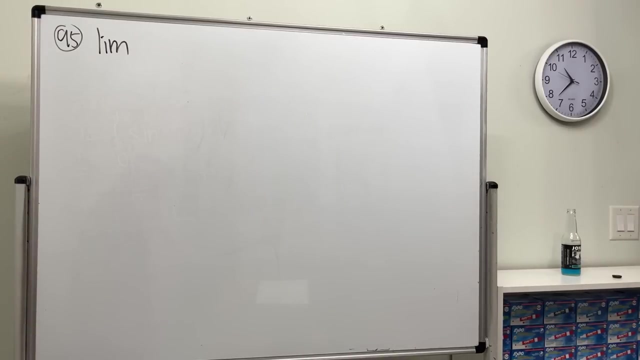 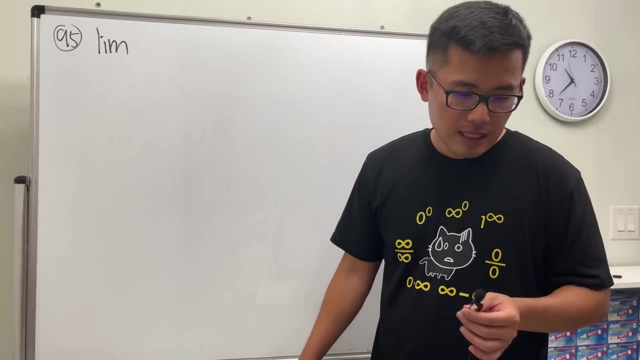 It's better that way. So we have the limit. Let me just see, I don't know why. I just want to check. Wow, 7 hours. Oh my goodness, Seriously, Yeah, Limit, And we have n goes to infinity. 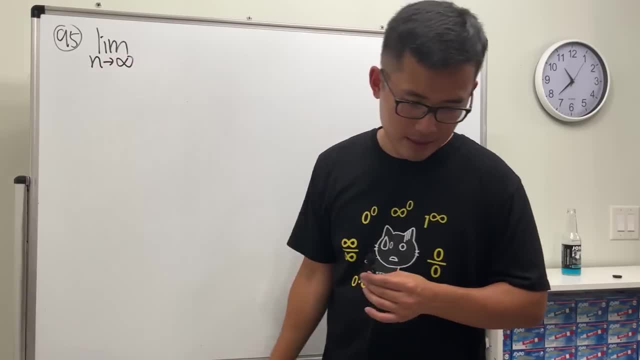 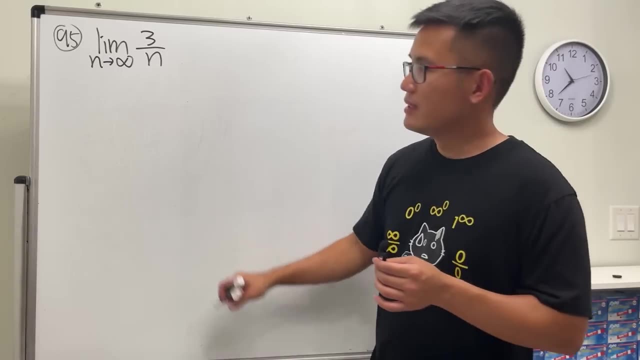 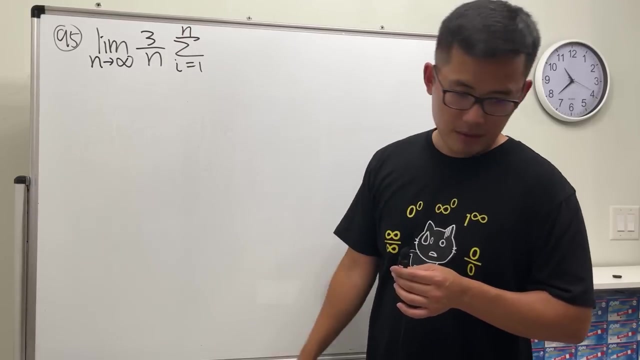 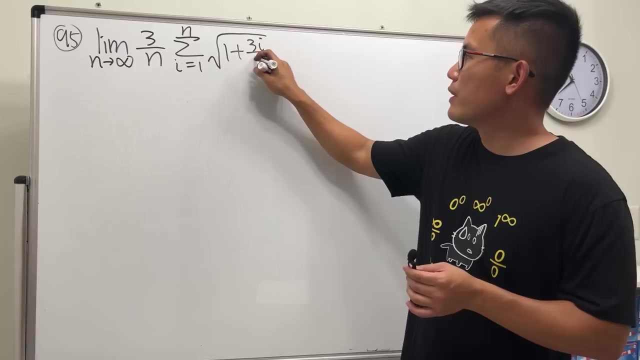 Yeah, of course n goes to infinity. What am I talking about? 3 over n And then times the summation, So I goes from 1 to n, Square root of 1 plus 3i over n. Wow, 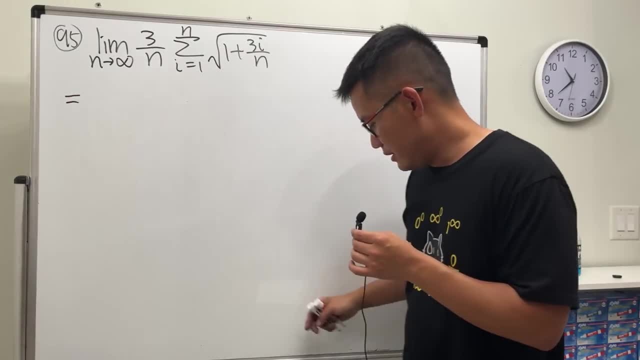 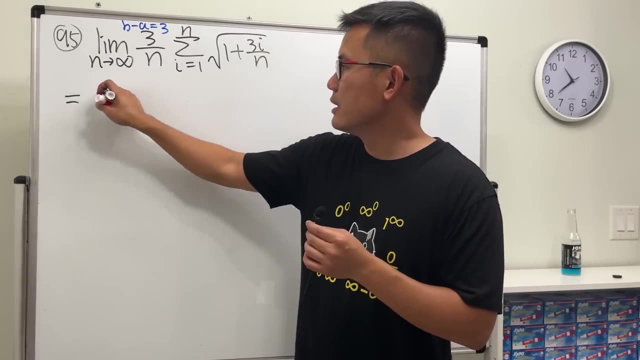 So how do we do this? First thing, first: 3, right b minus a is 3.. Just start with 0,. yeah, 0 to 3.. And this right here will give you the What's the function. 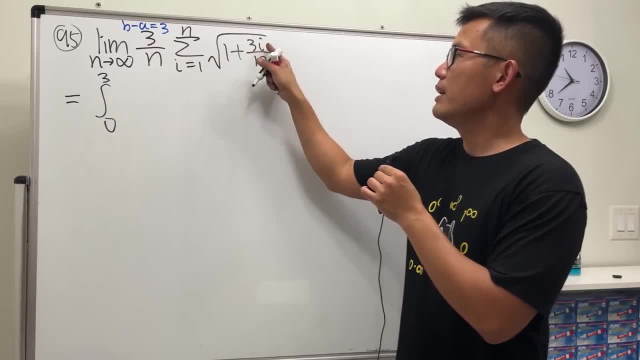 What's the function? What's the function? 3 and 3 match, So you pick the whole thing to be the x. So just square root of 1 plus x, Just like that. Work this out real quick, yeah, Okay. 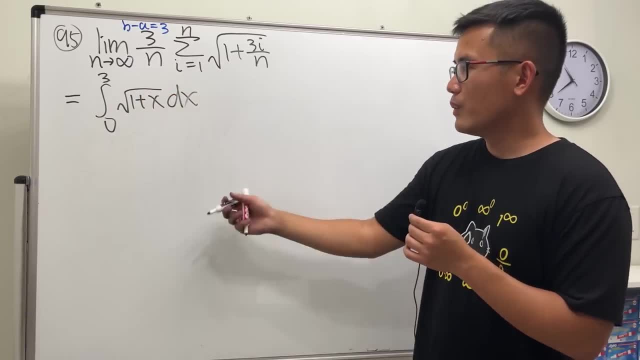 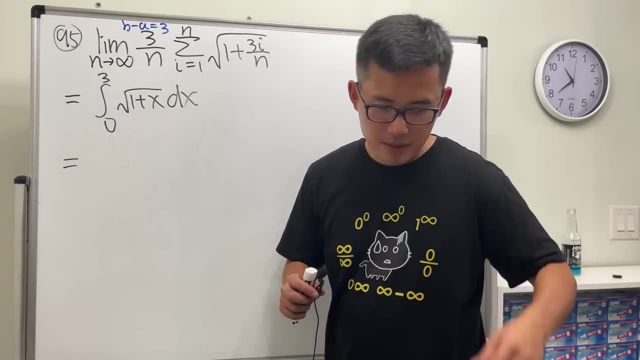 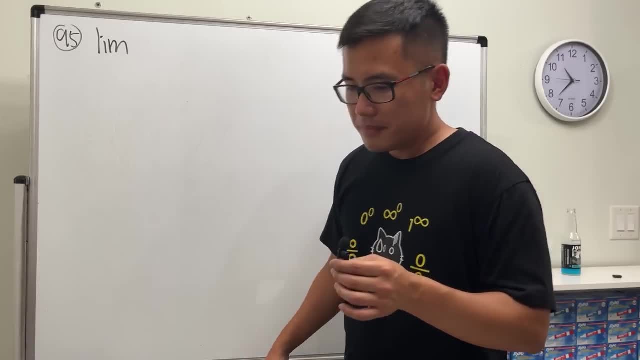 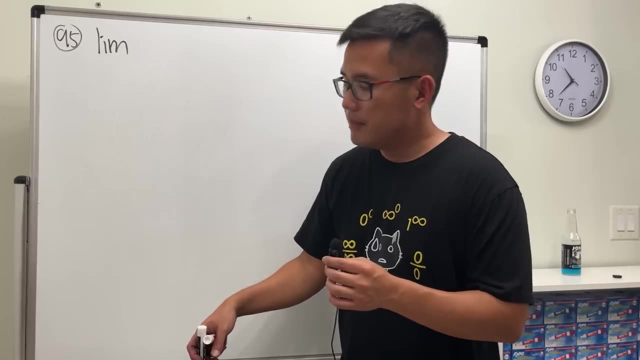 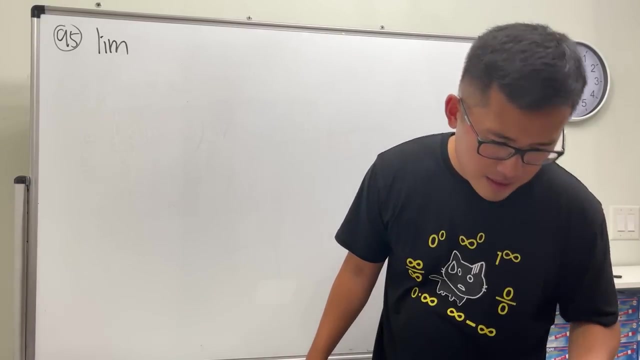 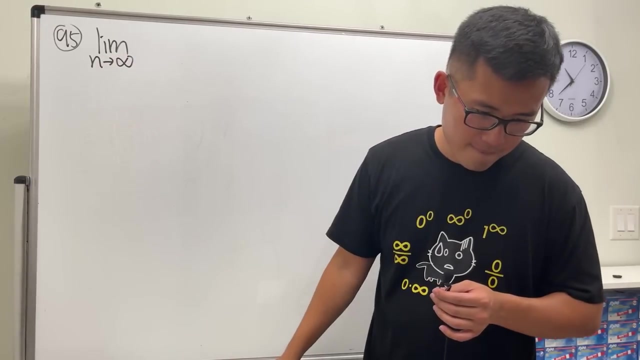 want to check, wow, seven hours. want to check, wow, seven hours? oh my goodness, oh my goodness, oh my goodness. seriously, yeah, yeah, yeah, limit and we have n goes to infinity. yeah, of course n goes. n goes to infinity. yeah, of course n goes. n goes to infinity. yeah, of course n goes to infinity. what am i talking about? 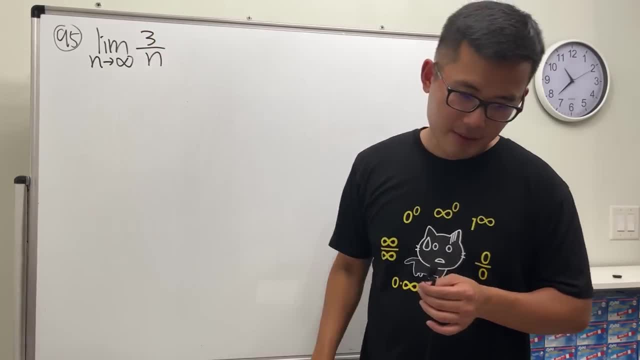 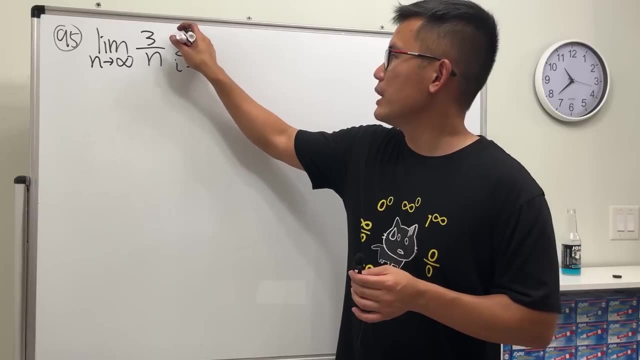 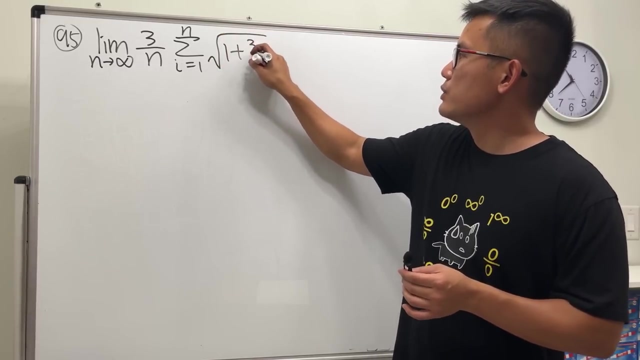 three over n, and then three over n, and then three over n, and then times the summation, times the summation, times the summation. i goes from one to n: square root of one plus three. i square root of one plus three. i square root of one plus three, i over n. whoa. 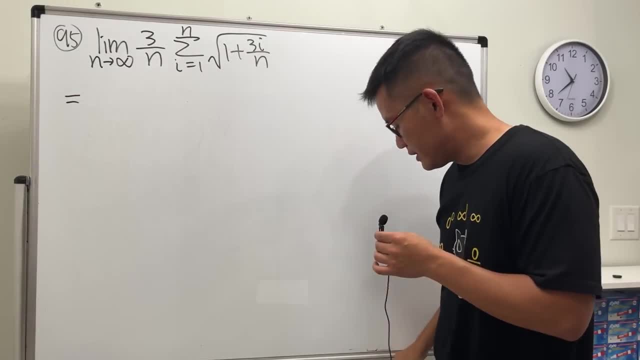 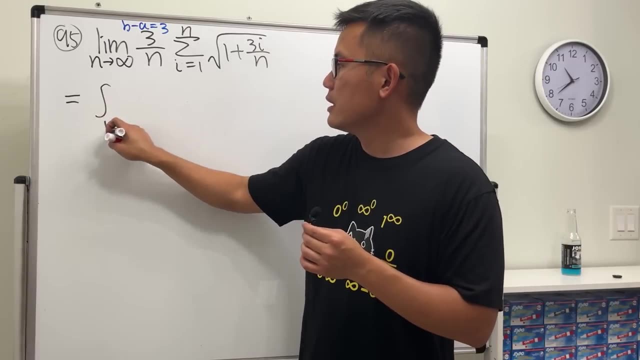 so how to do this first thing first. so how to do this first thing first. so how to do this first thing first: three right b minus a is three. three right b minus a is three. three right b minus a is three. just start with zero. yeah, just start with zero, yeah. 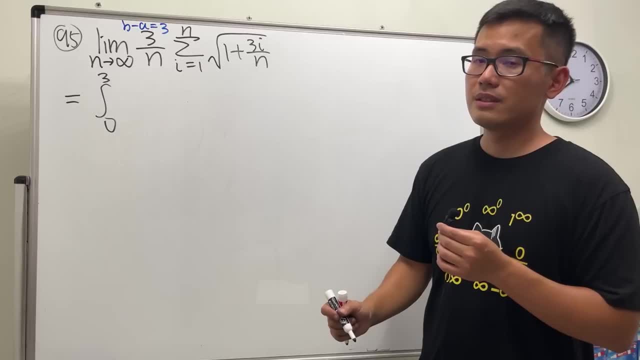 just start with zero. yeah, zero to three, and this right here will give zero to three, and this right here will give zero to three, and this right here will give you the function, you the function, you the function. what's the function, though? what's the function though? 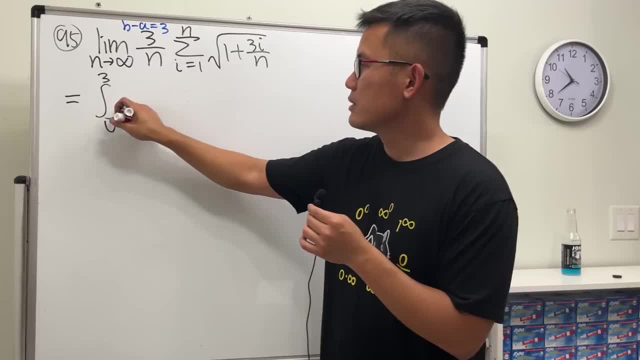 what's the function though? three and three match. so you pick the three and three match. so you pick the three and three match. so you pick the whole thing to be the x, whole thing to be the x, whole thing to be the x. so just square root of one plus x. 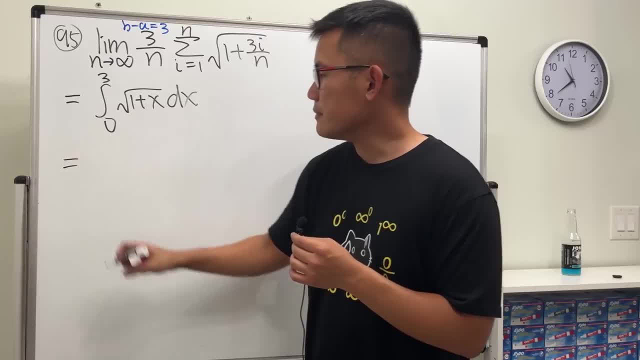 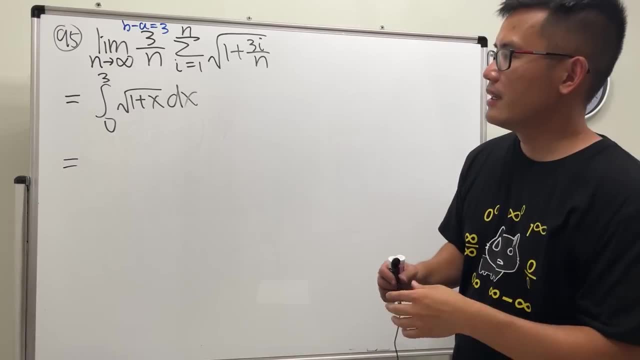 so just square root of one plus x. so just square root of one plus x, just like that. just like that, just like that. work this out real quick. yeah, work this out real quick. yeah, work this out real quick. yeah, uh, okay, okay, okay to do this right here. 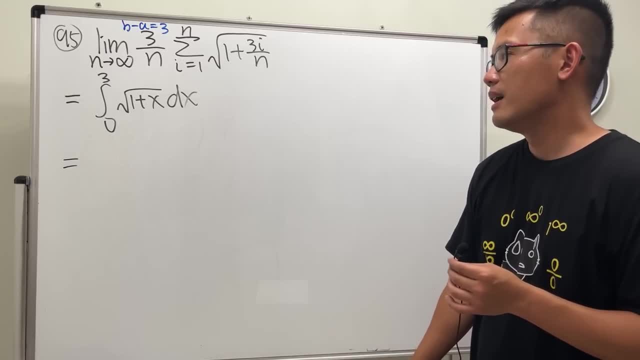 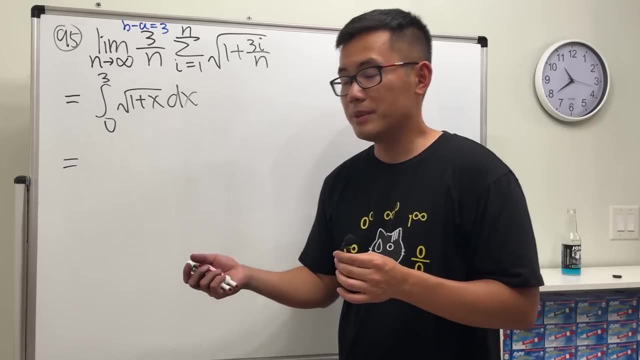 to do this right here. to do this right here, a okay, okay, this right here might not be the easiest. okay, this right here might not be the easiest. okay, this right here might not be the easiest to integrate at the moment. to integrate at the moment. 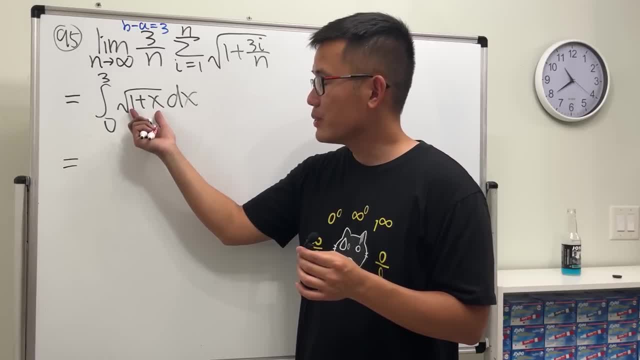 to integrate. at the moment, what we can do is right here inside. what we can do is right here inside. what we can do is right here inside. i'm just going to, i'm just going to, i'm just going to: minus one, minus one, minus one. i'm just going to move it. 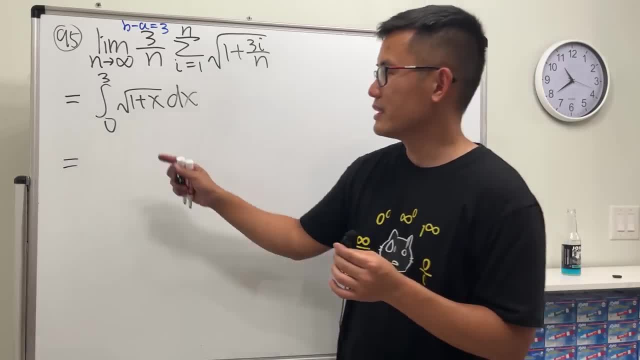 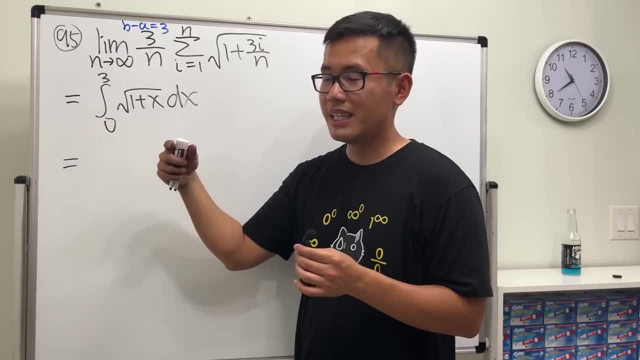 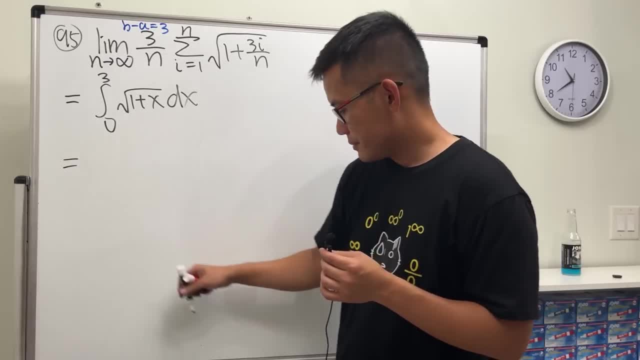 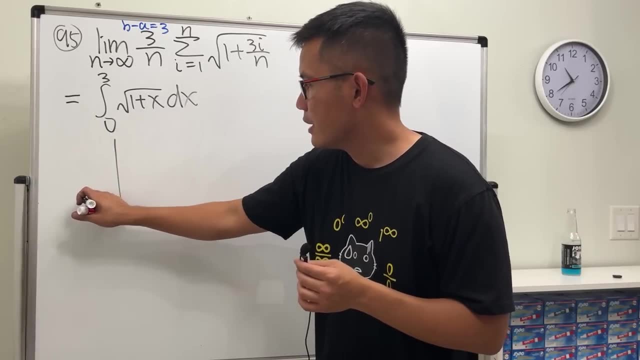 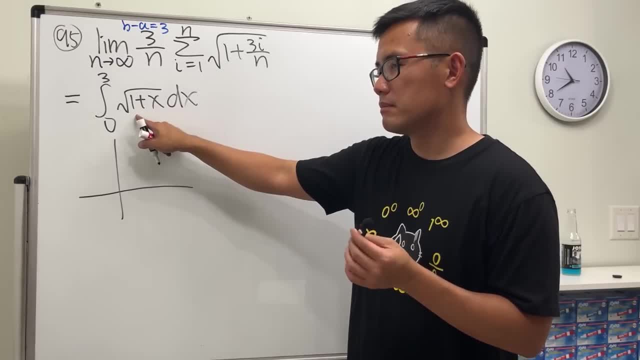 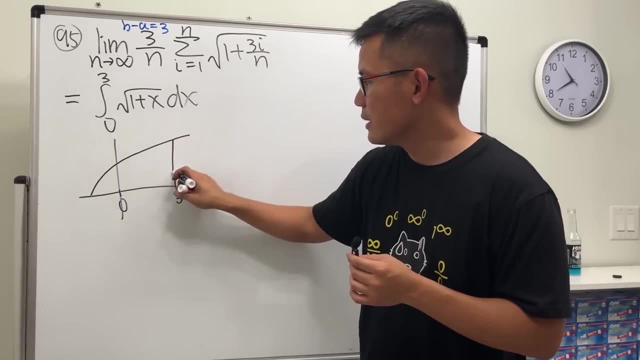 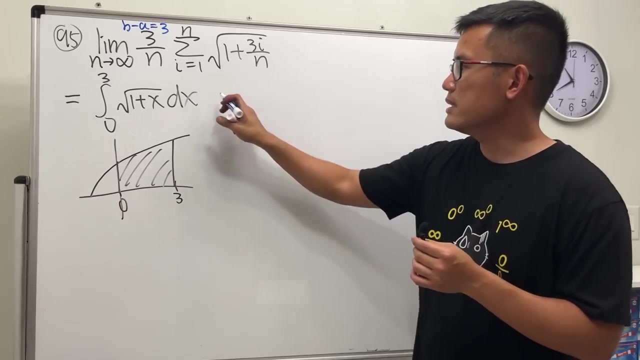 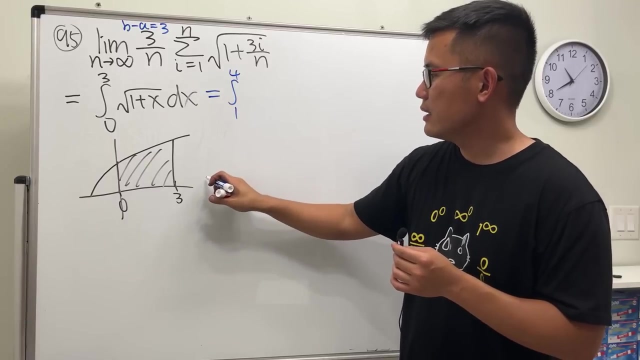 anyway, i'll send you so many times. anyway, this picture is like this: okay, and we go from zero to three, okay, but the truth is we can move it to the right one unit and that will give us the integral going from one to four, and then you can see that it's just. 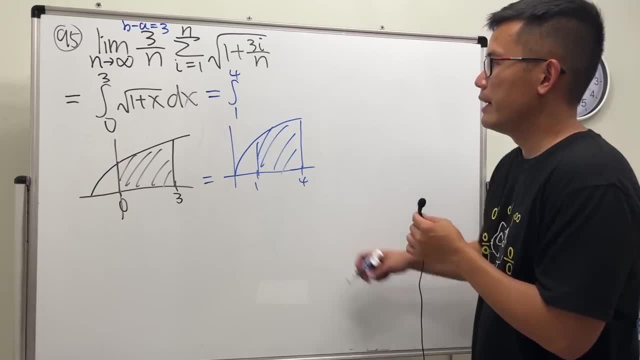 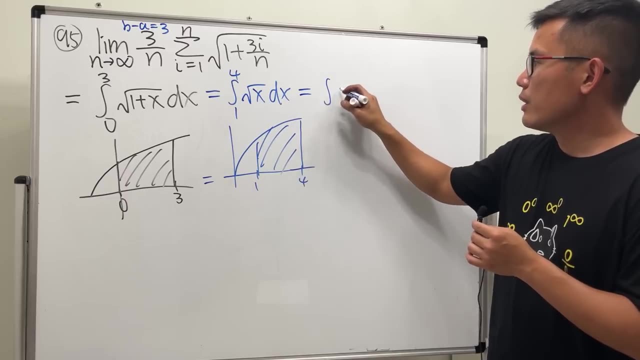 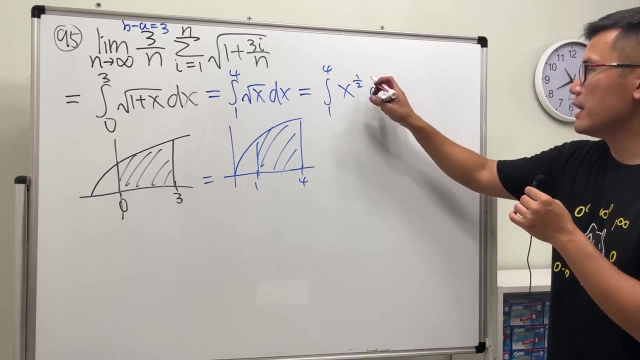 like this: it's the same area, okay, and we can just look at the square root of x, much easier to integrate, because now we can look at this as integral x to the one half power, dx one to four, and then just do the entire derivative that i showed you. i went to the power which is three half divided by the new power. 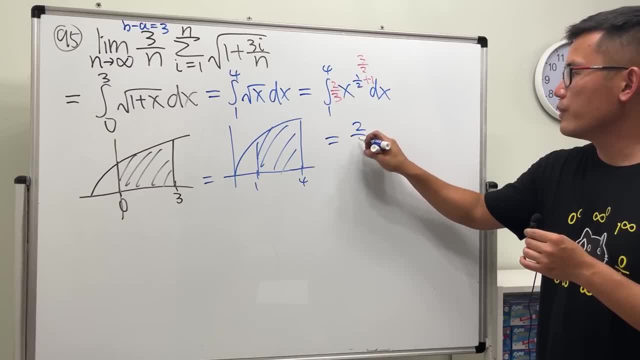 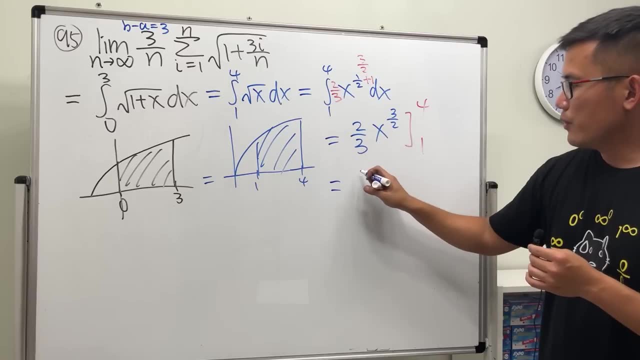 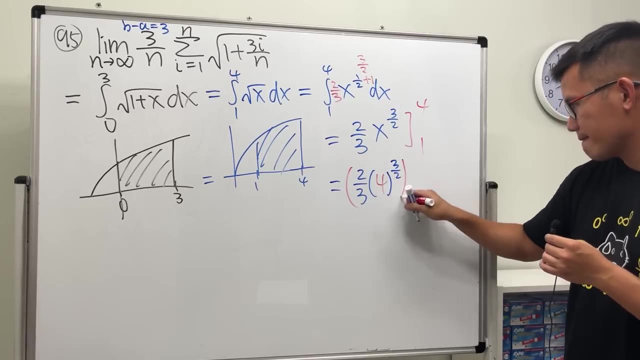 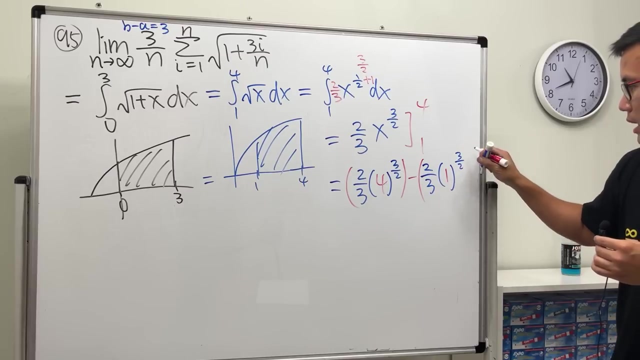 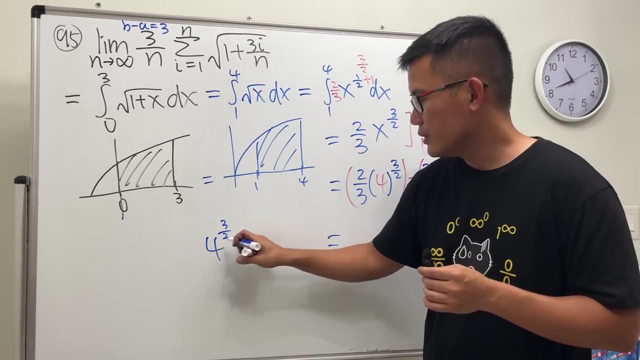 which is two over three, and this right here is two over three, x to this three over two, and then plug in, plug in here, putting the four and then putting the one, putting the one. okay, okay, four to these three over two is you take the square root of four first and then you. 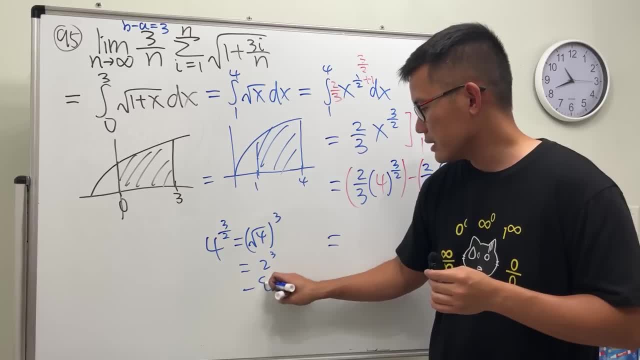 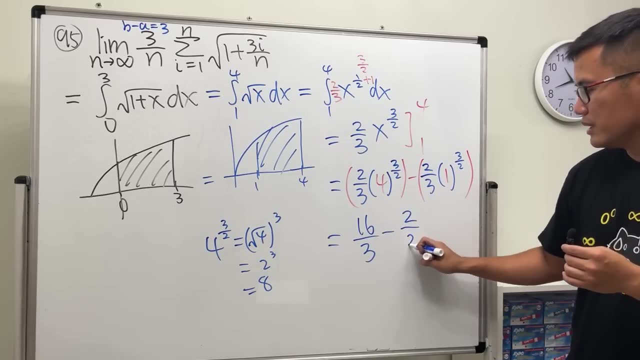 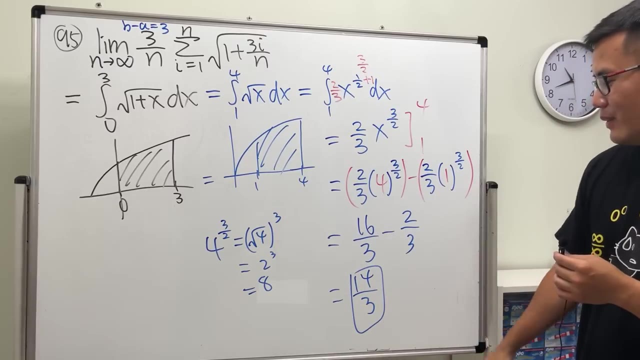 do the third power, which is two, to the third power, which is eight. so it's eight times that, which is sixteen over three. this is one, so it's minus two over three, so i know, fourteen over three, it's almost like pi, but the other way around. huh, wait, this is actually four point. 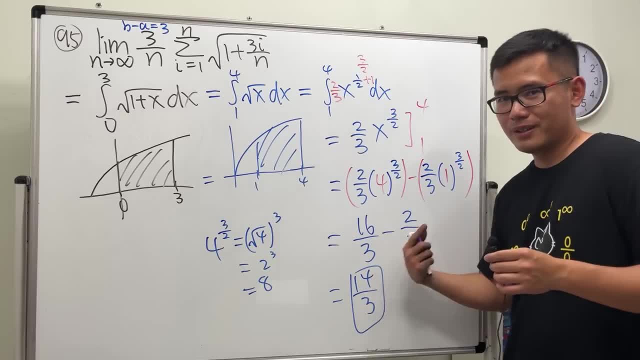 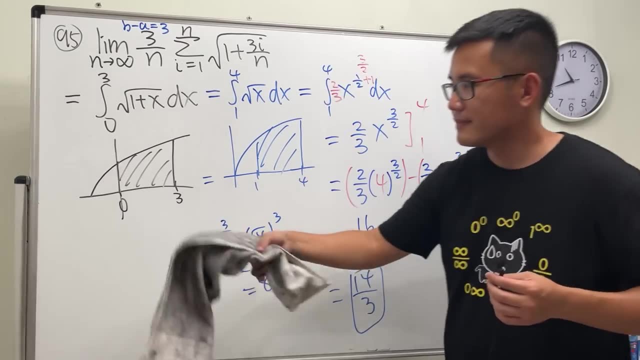 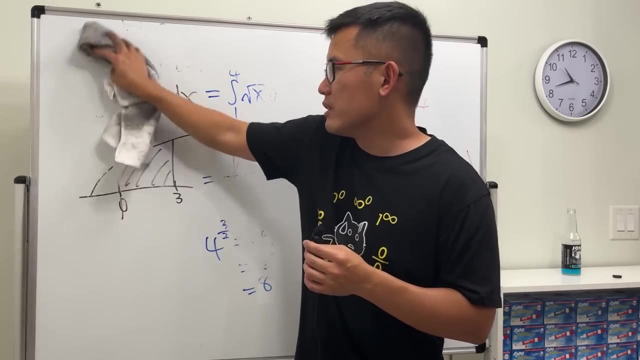 no, it's not. no, sorry. yeah, three, one, four. it's pretty upside down. by the way, that will be easier, okay. so it does have the advantage if you don't start with zero sometimes. but like that's um, if you just want to get a region, then start with zero much easier, and then, especially if you 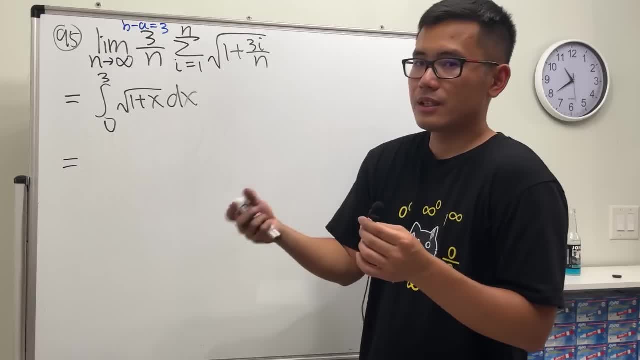 i'm just going to move it. i'm just going to move it, and then here i'm just going to add one, and then here i'm just going to add one, and then here i'm just going to add one. this is the same idea like shifting, okay. 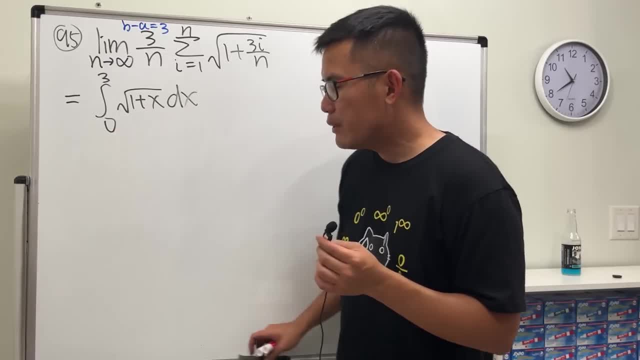 this is the same idea like shifting okay. this is the same idea like shifting okay, but anyway, but anyway, but anyway. i'll give you guys the area argument. i. i'll give you guys the area argument. i. i'll give you guys the area argument i. i think that's much better, okay. so here. i think that's much better okay. so here, i think that's much better okay. so here: yeah, because i don't want to get into yeah, because i don't want to get into yeah, because i don't want to get into the u substitution thing in this video. 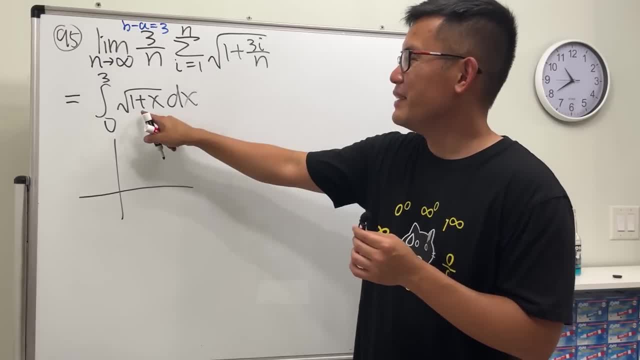 the u substitution thing in this video, the u substitution thing in this video. that's why, anyway, i said i knew so many. that's why, anyway, i said i knew so many. that's why, anyway, i said i knew so many times, times, times, anyway, anyway, anyway, this picture is like this: 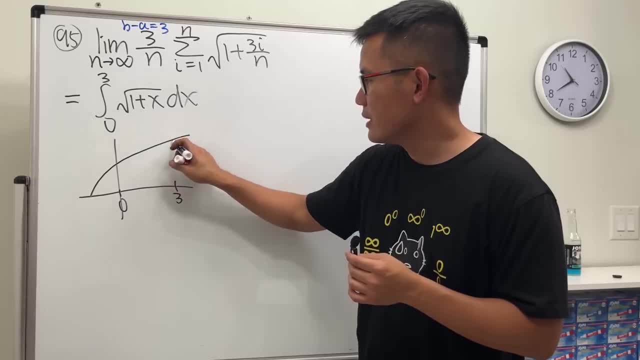 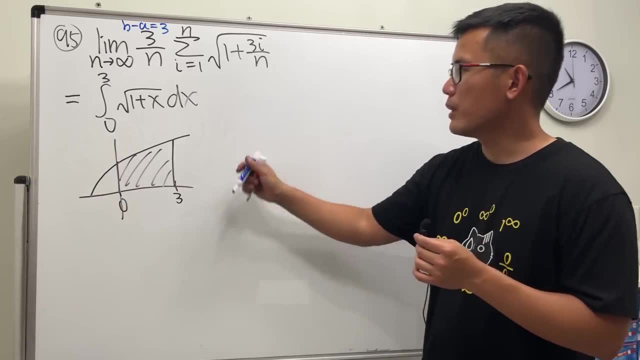 this picture is like this. this picture is like this: okay, and we go from zero to three, okay, okay, okay. but the truth is we can move it to the. but the truth is we can move it to the. but the truth is we can move it to the right one unit and that will give us the. 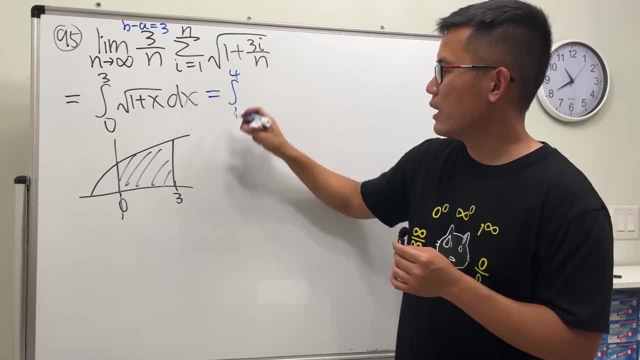 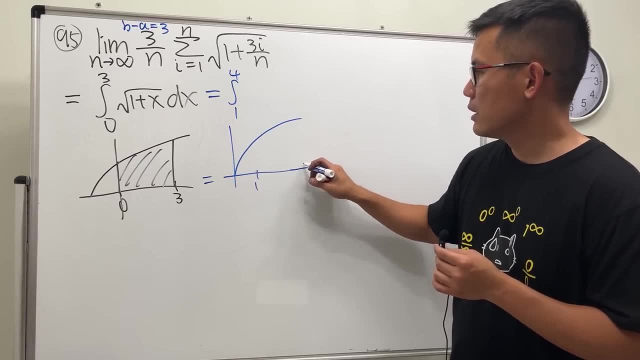 right one unit and that will give us the right one unit and that will give us the integral going from one to integral, going from one to integral, going from one to four, four, four and then, and then, and then. you can see that, you can see that, you can see that it's just. 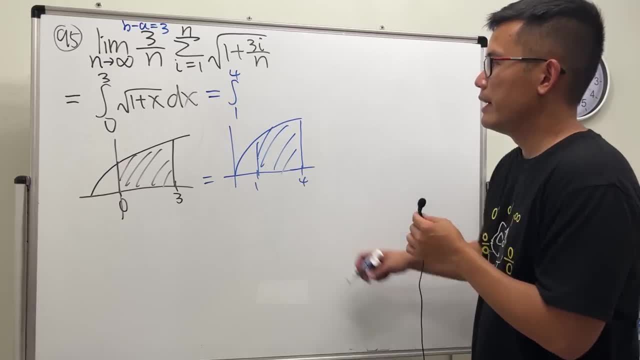 like this: it's the same area. like this: it's the same area. like this, it's the same area. okay, okay, okay, and we can just look at the square root, and we can just look at the square root, and we can just look at the square root of x. 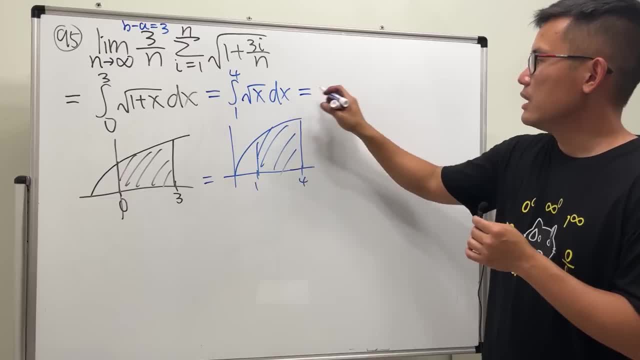 of x, of x much easier to integrate, because now we much easier to integrate, because now we much easier to integrate, because now we can look at this, as can look at this, as can look at this as integral x to the one half power dx. integral x to the one half power dx. 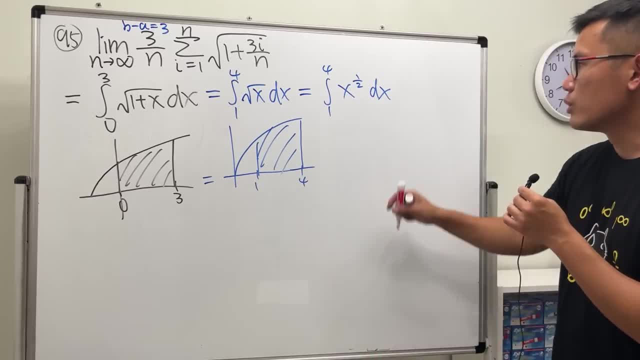 integral x to the one half power, dx one to four, and then one to four, and then one to four, and then just do the entire derivative, that i just do the entire derivative, that i just do the entire derivative that i showed you, showed you, showed you, i went to the power, which is three half. 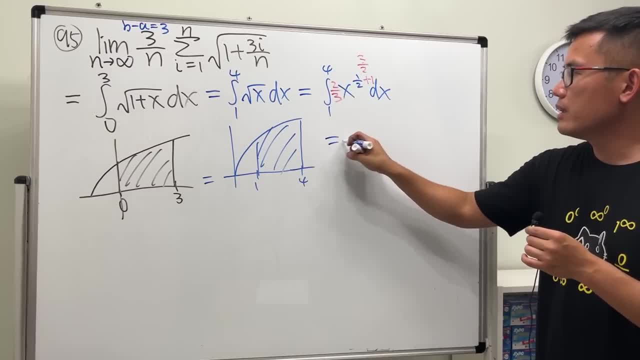 i went to the power which is three half. i went to the power which is three half, divided by the new power, which is two, divided by the new power, which is two, divided by the new power, which is two over three. and this right here is over three and this right here is. 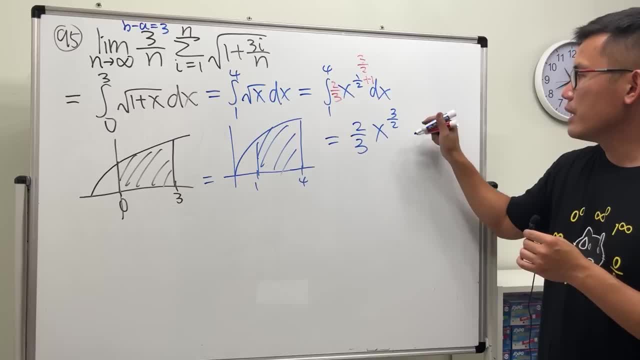 over three, and this right here is: two over three, x to these three over two, two over three, x to these three over two, two over three, x to these three over two, and then plug in, plug in here and then plug in, plug in here and then plug in, plug in here, put in the four and then put in the. 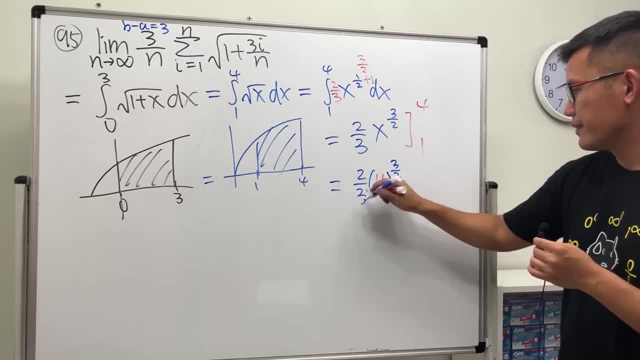 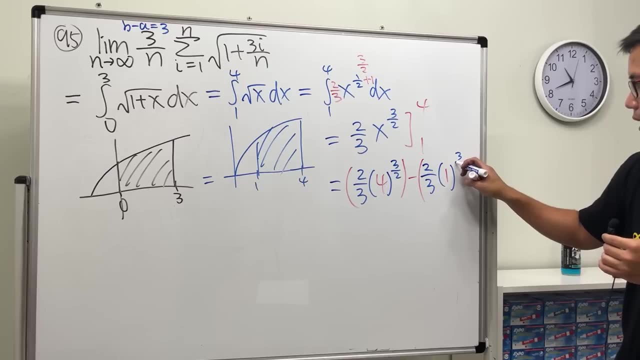 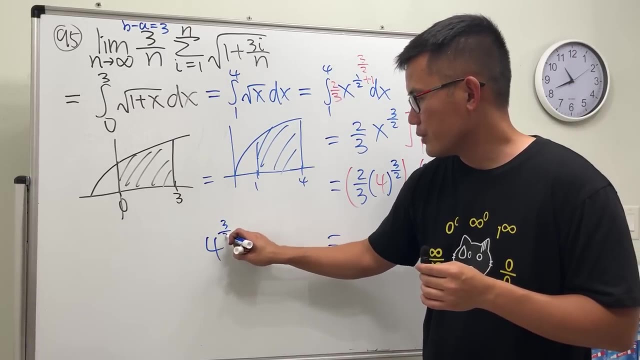 put in the four and then put in the. put in the four and then put in the one. putting the one. okay, okay, okay, okay, okay, okay. four to these three over two. is you take four to these three over two? is you take four to these three over two? is you take the square root of four first and then? 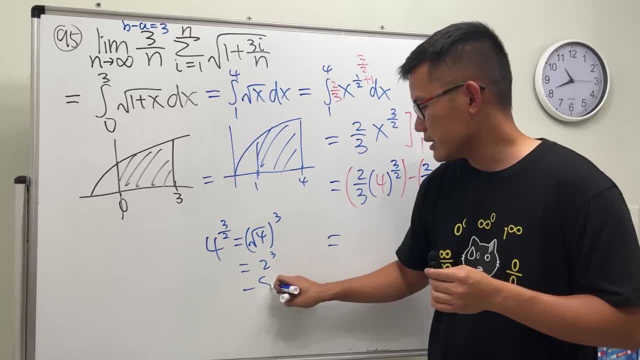 the square root of four first, and then the square root of four first, and then you do the third power, which is two to, you do the third power, which is two to, you do the third power which is two to the third power, which is eight, the third power, which is eight. 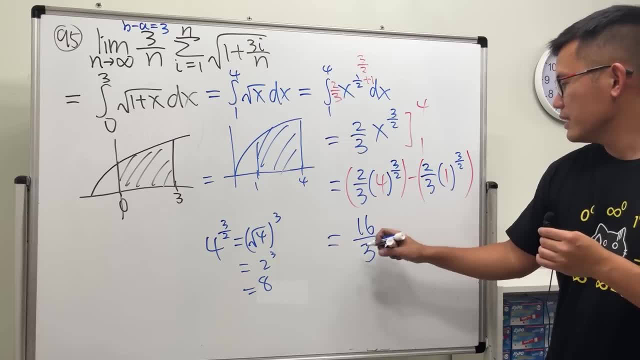 the third power, which is eight, so it's eight times that, which is six, so it's eight times that which is six, so it's eight times that which is six. 16 over three: this is one, so it's minus. 16 over three: this is one, so it's minus. 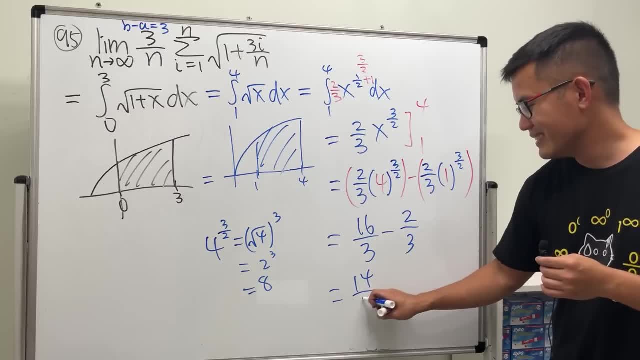 16 over three. this is one, so it's minus two over three. so i know two over three, so i know two over three. so i know 14 over three it's almost like pi. but 14 over three it's almost like pi. but 14 over three it's almost like pi, but the other way around, huh. 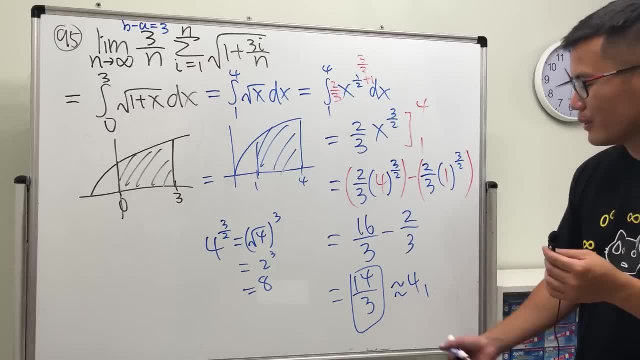 the other way around. huh, the other way around. huh. wait, this is actually four point. wait, this is actually four point. wait, this is actually four point. no, it's not, no, sorry, yeah, three, one. no, it's not, no, sorry, yeah, three, one. no, it's not, no, sorry, yeah, three, one, four, it's pretty upside down. 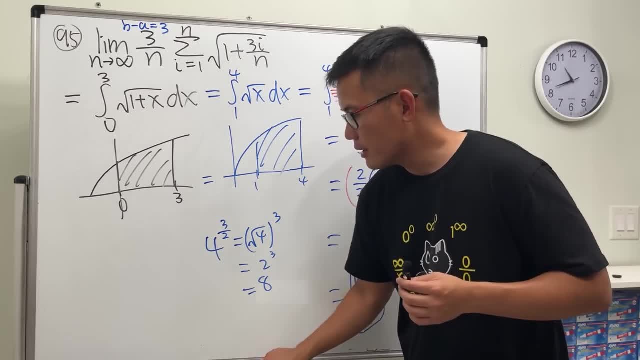 four, it's pretty upside down. four, it's pretty upside down, by the way. that will be easier by the way. that will be easier by the way. that will be easier. okay, okay, okay. so it does have the advantage if you. so it does have the advantage if you. 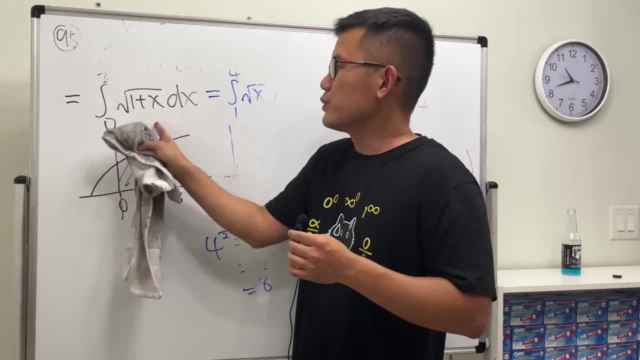 so it does have the advantage if you don't start with zero sometimes, but like don't start with zero sometimes, but like don't start with zero sometimes, but like that's, that's, that's if you just want to get a region, then if you just want to get a region, then 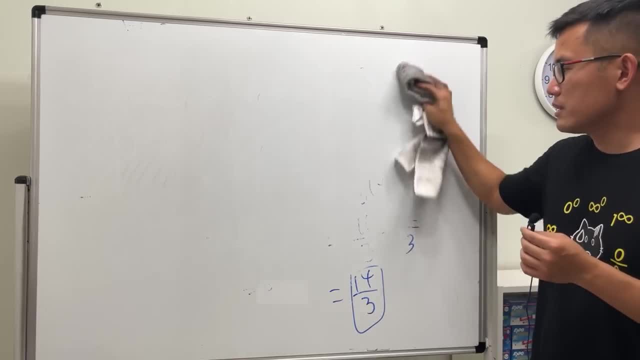 if you just want to get a region, then start with zero much easier, and then start with zero much easier, and then start with zero much easier. and then, especially if you are familiar with how, especially if you are familiar with how, especially if you are familiar with how to do the integral, that you can do the 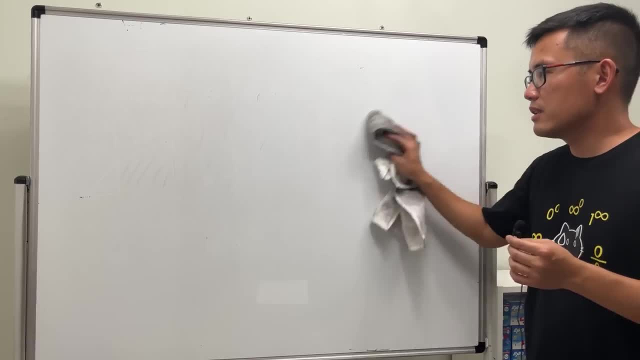 to do the integral that you can do, the, to do the integral that you can do, the so-called u substitution, so-called u substitution, so-called u substitution, or some kind of magic, and then you can, or some kind of magic, and then you can, or some kind of magic, and then you can figure out the answer one way or the. 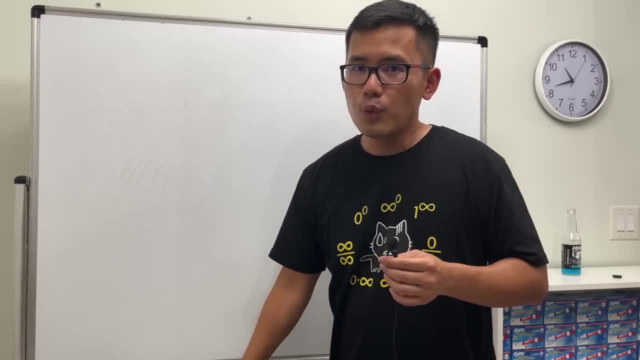 figure out the answer one way or the figure out the answer one way or the other. i wonder what if i don't do? i wonder what if i don't do. i wonder what if i don't do? all 100 questions. is there anybody who's all 100 questions? is there anybody who's? 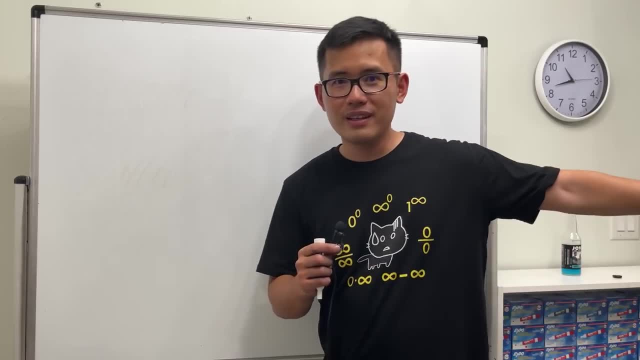 all 100 questions. is there anybody who's going to notice, going to notice? going to notice. if you have watched the whole thing, if you have watched the whole thing, if you have watched the whole thing. definitely leave a comment down below. definitely leave a comment down below. 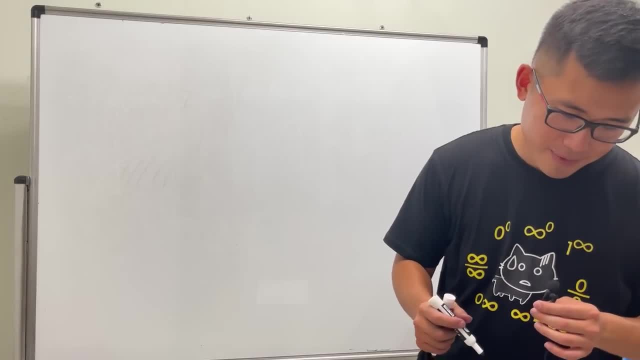 definitely leave a comment down below link, but don't lie, though. be honest. link, but don't lie, though. be honest. link, but don't lie, though, be honest. i'm, i'm, i'm, i did the whole thing. i did the whole thing. i did the whole thing, okay. 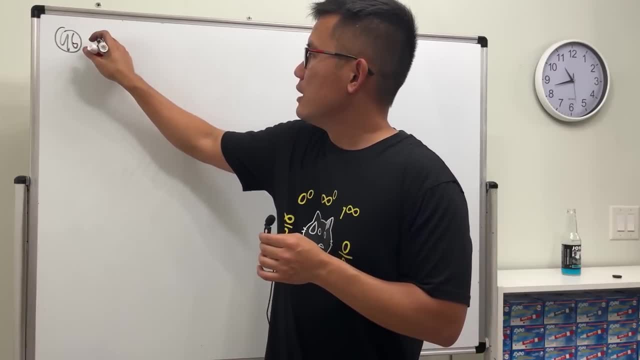 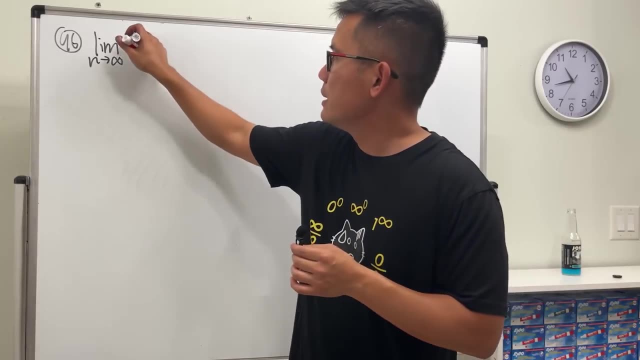 okay, okay, 97 no 96, 97 no 96, 97 no 96. limit limit limit: n goes to infinity, and then we have n goes to infinity, and then we have n goes to infinity, and then we have one over n, one over n, one over n sum. 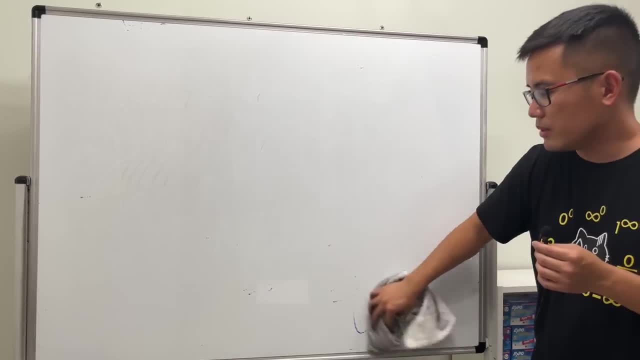 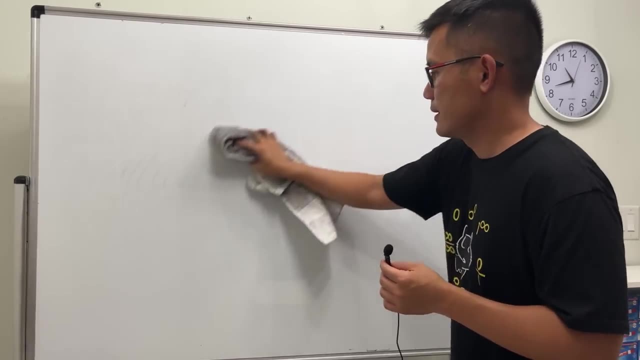 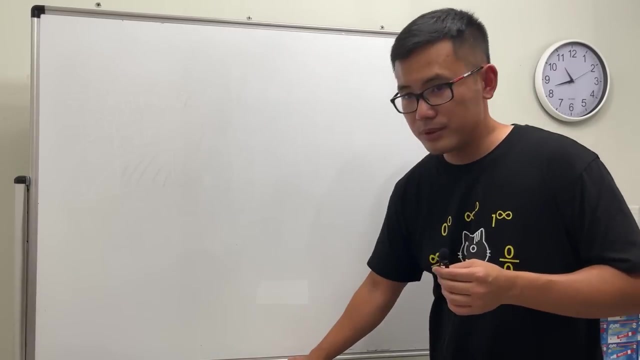 are familiar with how to do the integral, that you can do the so-called use, substitution or some kind of magic, and then you can figure out the answer. i wonder what if i don't do all 100 questions. is there anybody who's going to notice? if you have watched the whole thing, definitely leave a comment down below link, but don't. 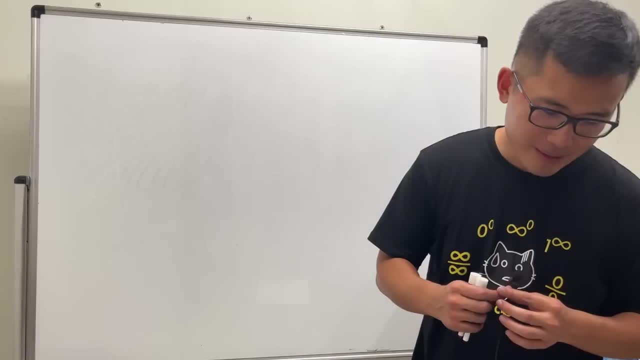 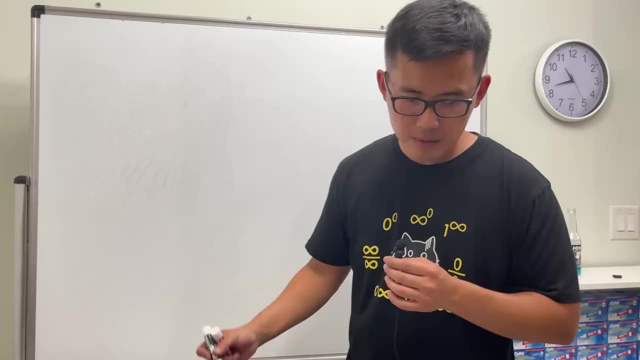 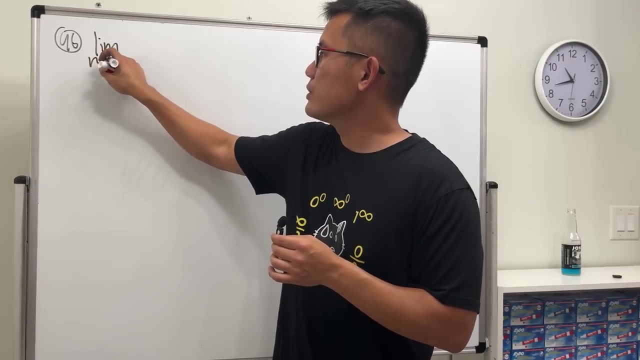 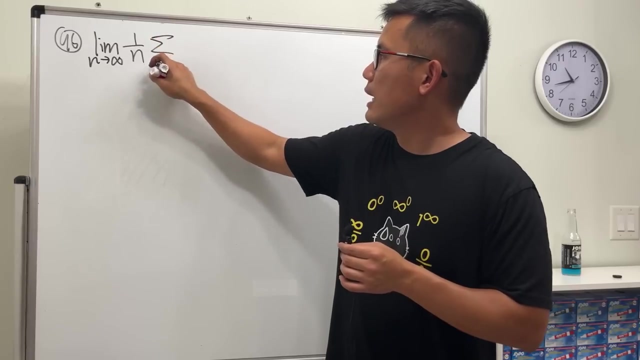 lie, though be honest. um, i did the whole thing, okay. 97, no, 96.. limit- i'm going to give you a little bit of an idea- goes to infinity, and then we have 1 over n sum. I goes from 1 to infinity and then 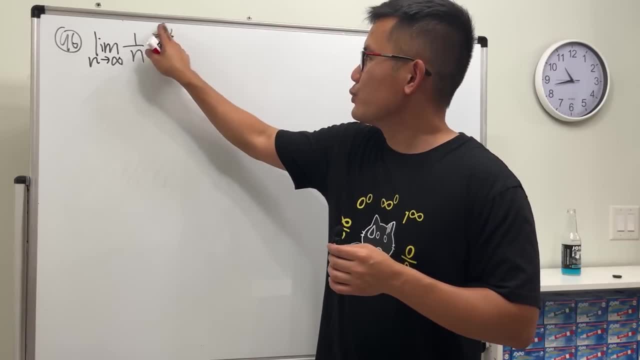 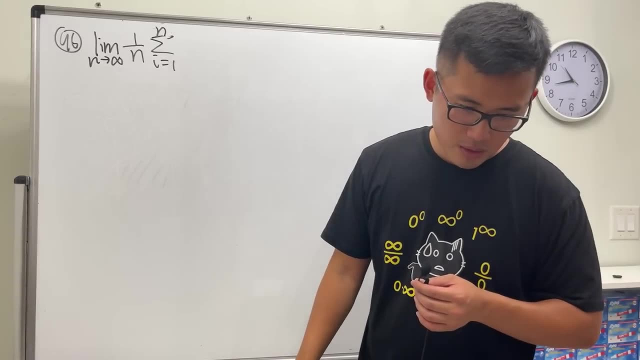 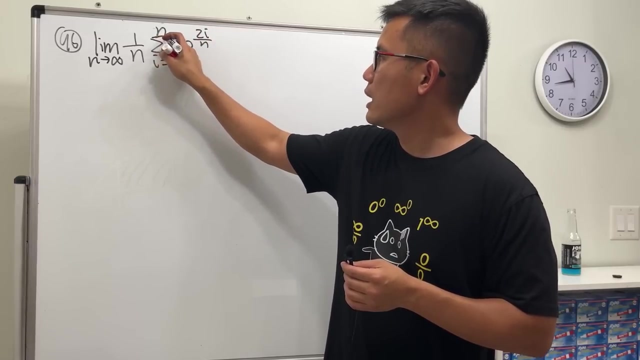 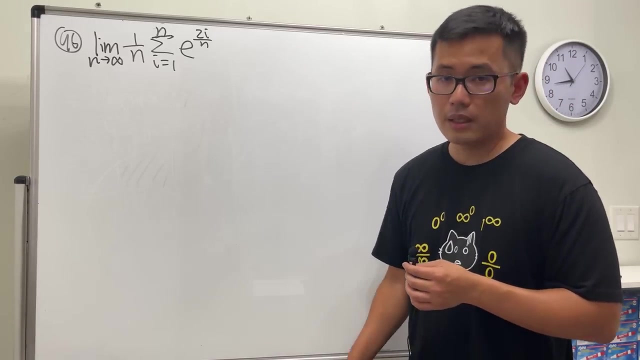 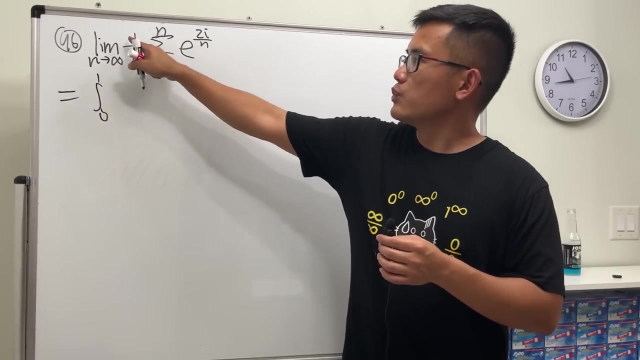 we have. no, no, no, no. I always want to write like Sigma down C to the infinity, because that's what we do in Cal 2 all the time. no e to the 2i over n power. okay, okay, ready, cool. it's 1 over n. so just integral going from 0 to 1 here. this is: 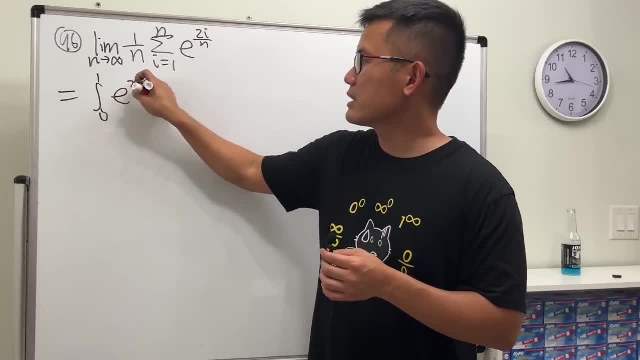 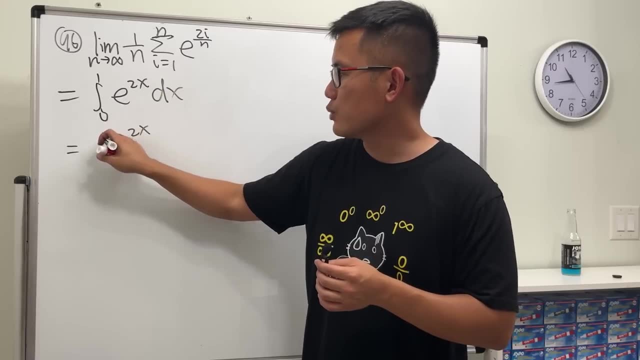 1. this is 2, so the function is e to the 2x. okay, integrate this. e to the 2x stays but divided by 2, because that's the derivative of 2x, and then just plug in numbers 0, 1. be really careful. 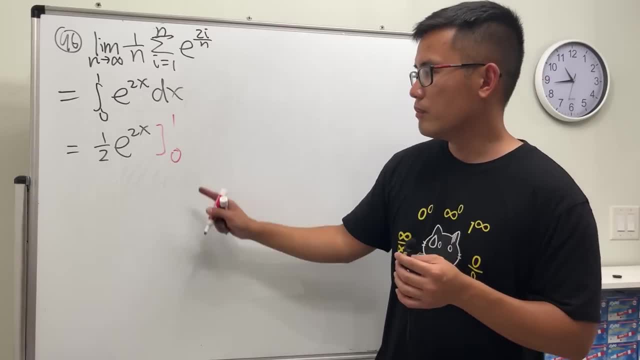 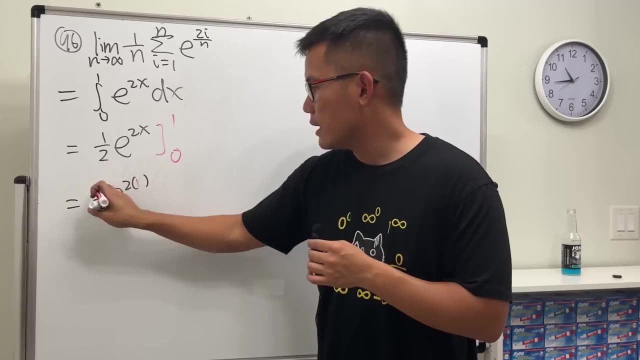 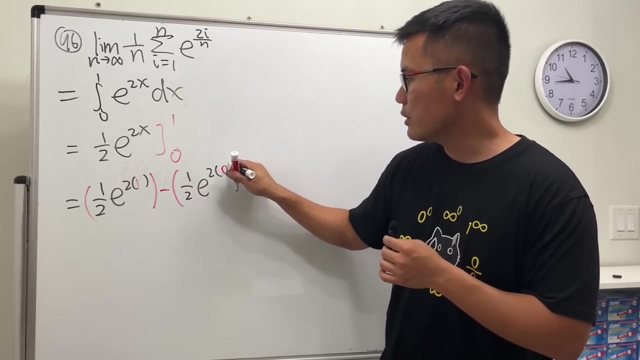 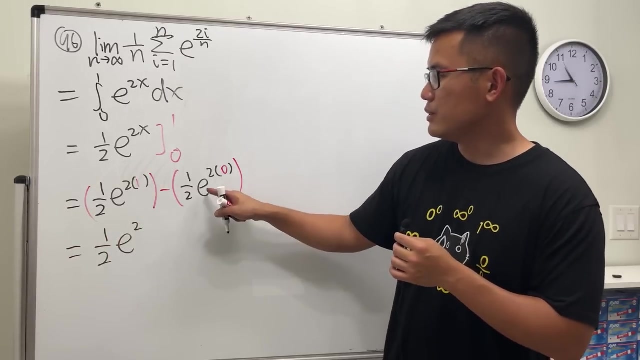 with when you plug in zeros. sometimes it does matter, so don't ignore it. so here we have: 1 half e to the 2 times 1 and then minus. plug in 0. 1 half e to the 2 times 0. okay, this is just 1 over 2 e square, and this is just 1, so just minus. 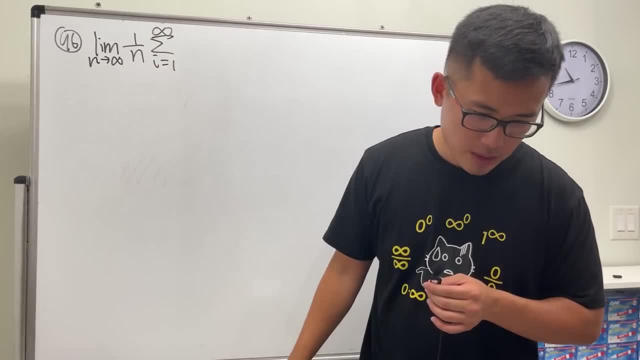 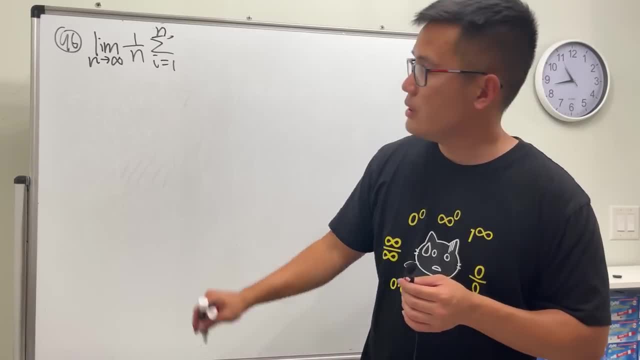 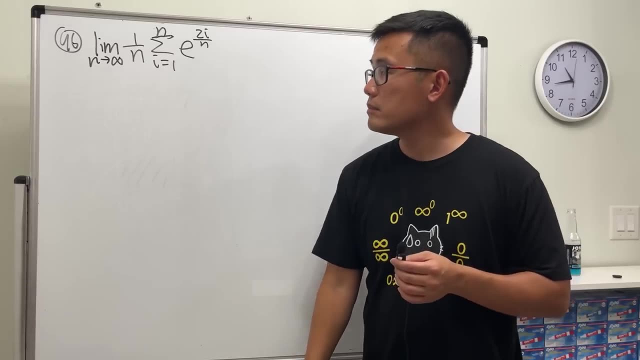 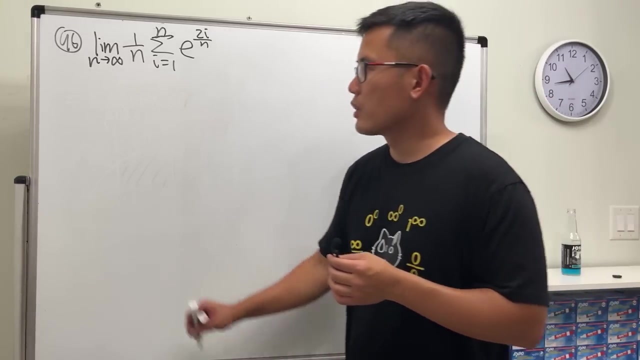 what we do in cal 2 all the time. but no, but no, but no. e to d, e to d, e to d, 2i over n's power, 2i over n's power, 2i over n's power. okay, okay, okay, okay, ready, cool. 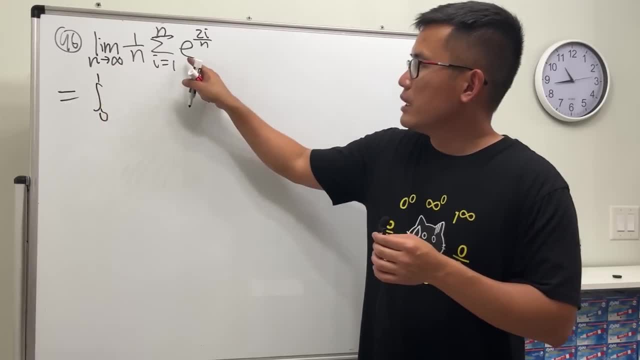 ready, cool, ready, cool. it's one over n, so just integral going. it's one over n, so just integral going. it's one over n, so just integral going from zero to one, from zero to one, from zero to one here, this is one, this is two, so 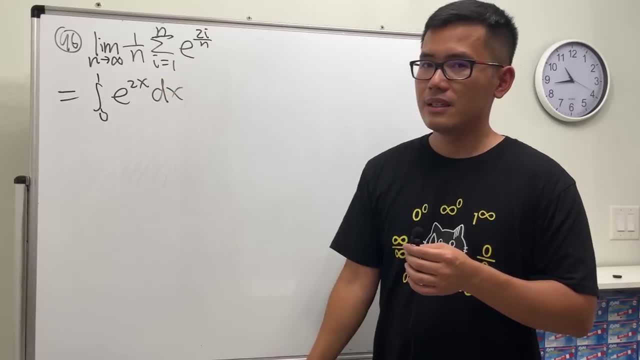 here, this is one, this is two. so here, this is one, this is two. so the function is e to the 2x, the function is e to the 2x. the function is e to the 2x. okay, okay, okay, integrate this, integrate this, integrate this. e to the 2x stays, but divided by 2. 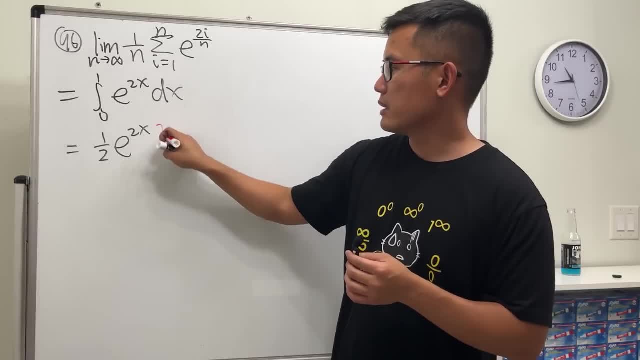 e to the 2x stays, but divided by 2. e to the 2x stays, but divided by 2, because that's the derivative of, because that's the derivative of, because that's the derivative of 2x, and then just plug in numbers zero and 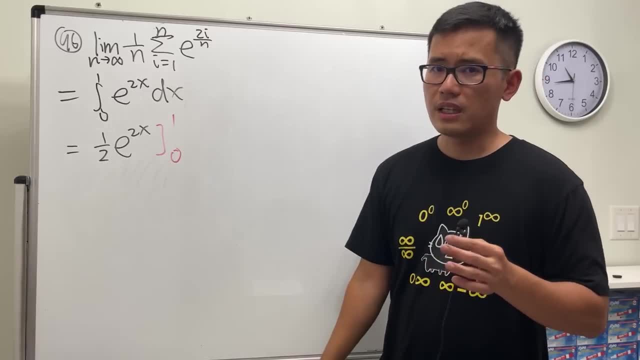 2x and then just plug in numbers zero and 2x and then just plug in numbers zero and one, one one. be really careful with when you plug in. be really careful with when you plug in. be really careful with when you plug in zeros. sometimes it does matter so. 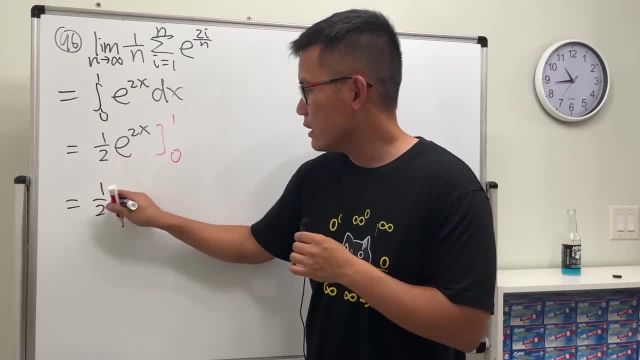 zeros, sometimes it does matter. so, zeros, sometimes it does matter. so don't ignore it, don't ignore it, don't ignore it. so here we have one half, so here we have one half, so here we have one half. e to the two times one, and then minus. 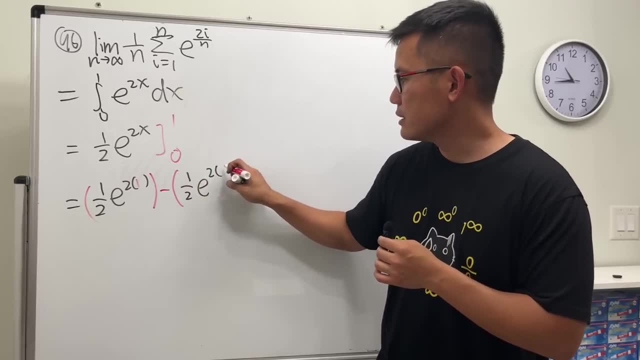 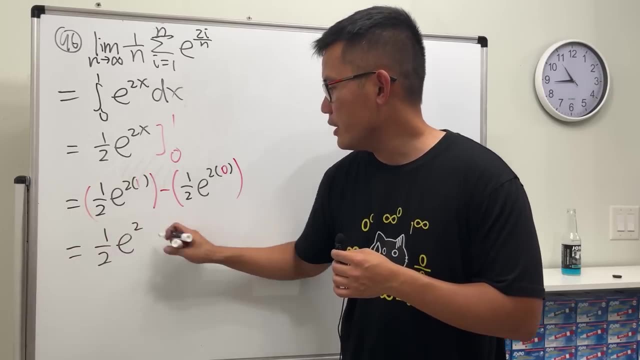 and then minus, and then minus. plugging zero: one half e to the two times plugging zero. one half e to the two times plugging zero. one half e to the two times zero. zero, zero, okay, okay, okay. this is just one over two e square. this is just one over two e square. 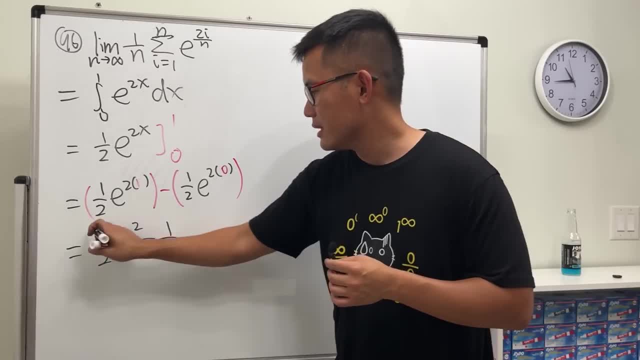 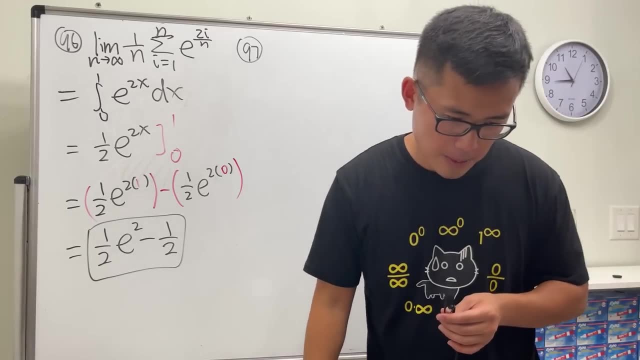 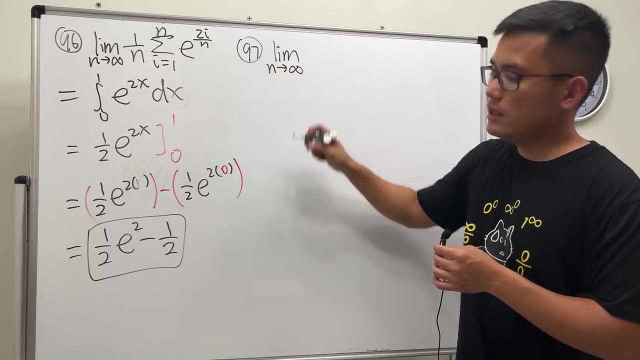 this is just one, over two e square, and this is just one, so just minus one. and this is just one, so just minus one. and this is just one, so just minus one. half half half, done, done, done, 97, okay, okay, okay. limit as n goes to infinity and we have. 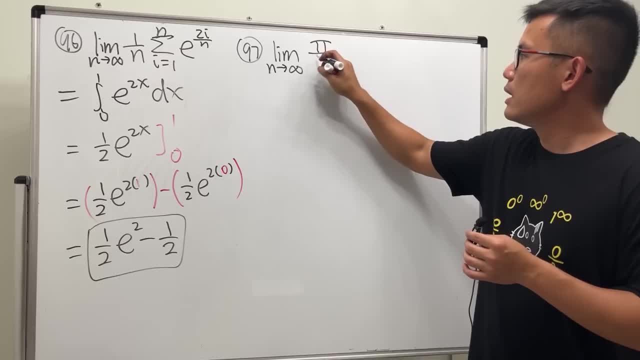 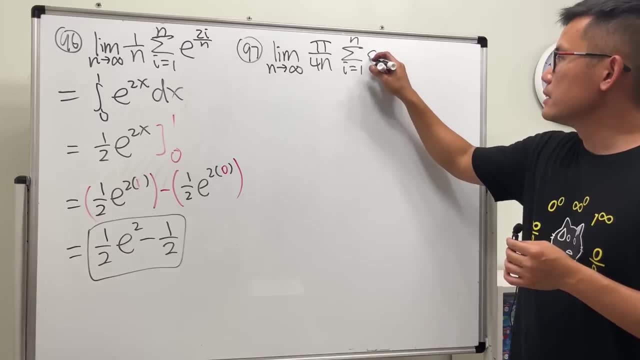 limit, as n goes to infinity, and we have limit, as n goes to infinity and we have pi over 4, n sum i goes from 1 to n and then sum i goes from 1 to n and then sum i goes from 1 to n and then secant square. 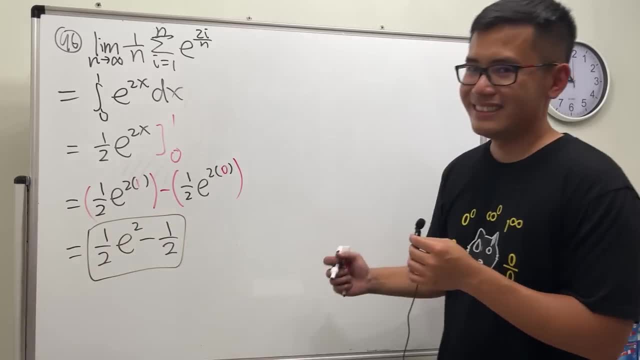 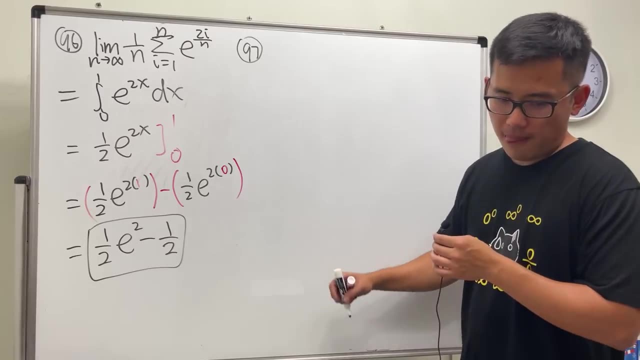 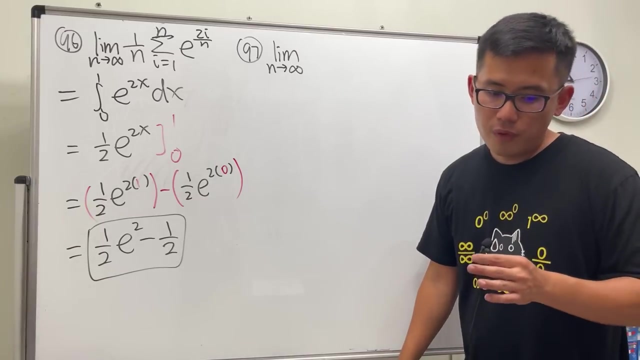 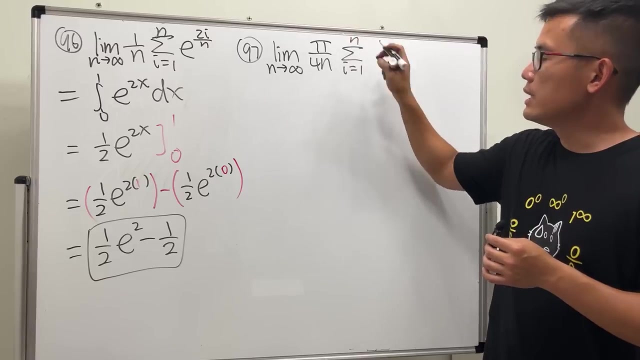 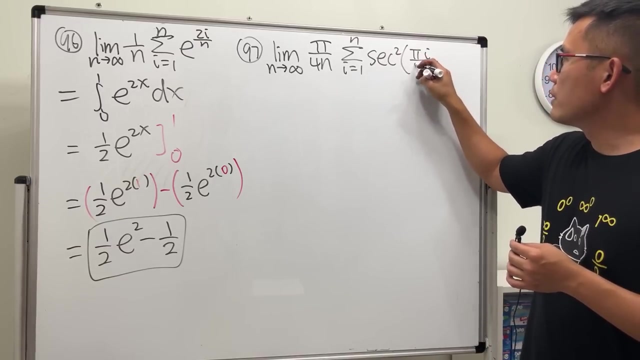 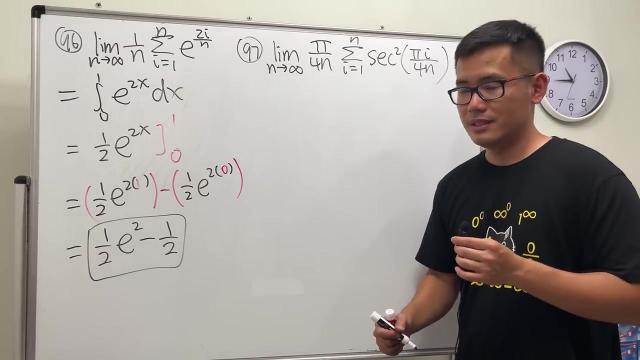 1 half, 1 half. okay limit as n goes to infinity. we have pi over 4 n. sum: I goes from 1 to n and then cm square: pi i over 4 n, pi over 4,, pi over 4, match: This means we go from 0 to pi over 4.. 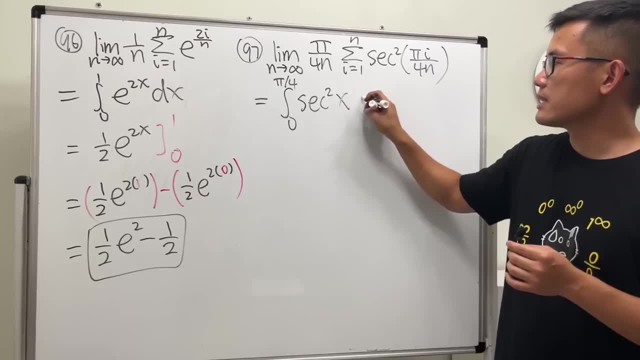 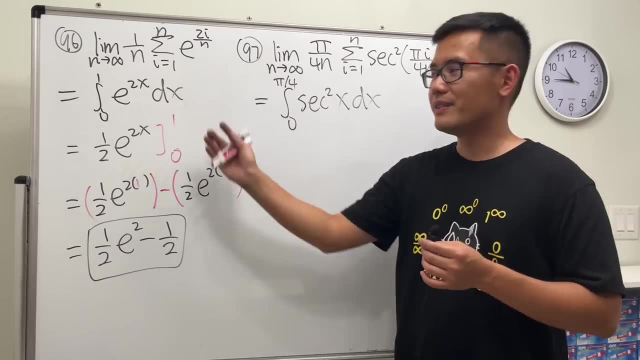 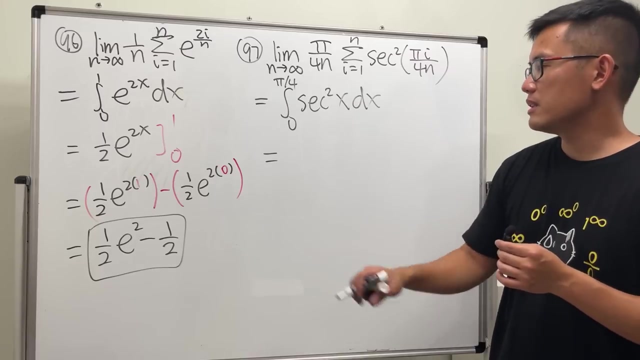 And the input is just what? secant squared x, dx, Okay, Yeah, Very different, Very different, Okay. and now let's just work this out: The derivative of what function will give us secant squared? The answer is tangent. 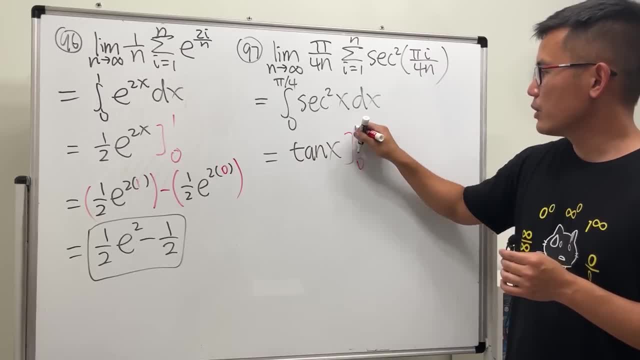 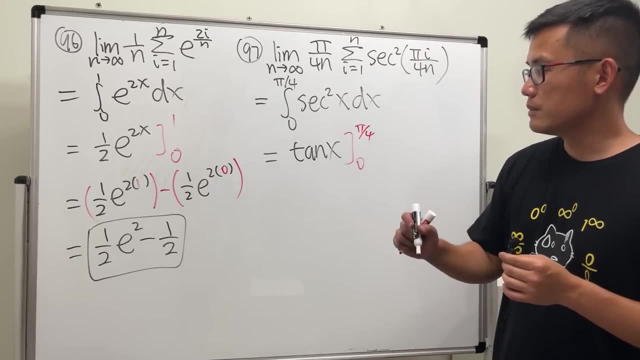 So tangent x 0, pi over 4.. Plugging pi over 4, tangent of pi over 4 is 1.. Plugging 0, tangent of 0 is 0. So all in all, the answer is just 1.. 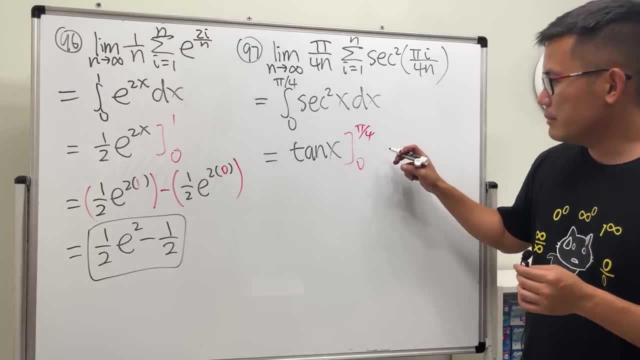 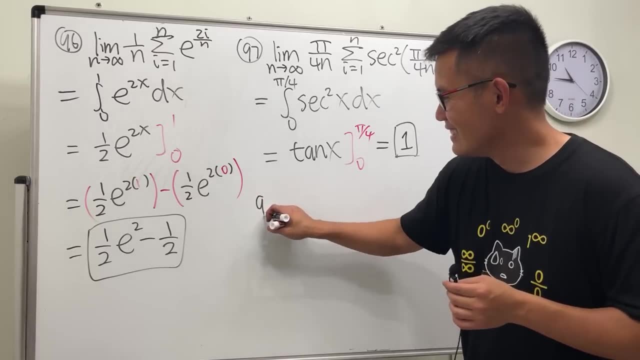 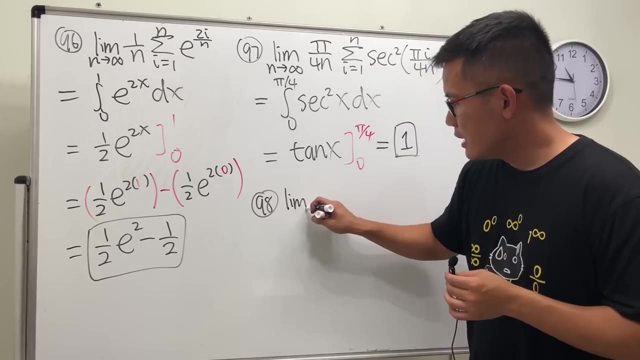 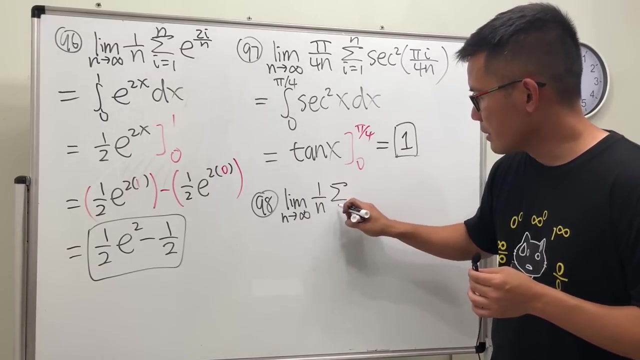 So nice, Yeah. so I'm just going to write it right here Because I want to fit another question here: Number 98.. Number 98.. Number 98.. Okay, Here's the limit, as n goes to infinity, And then we have 1 over n sigma. i goes from 1 to n. 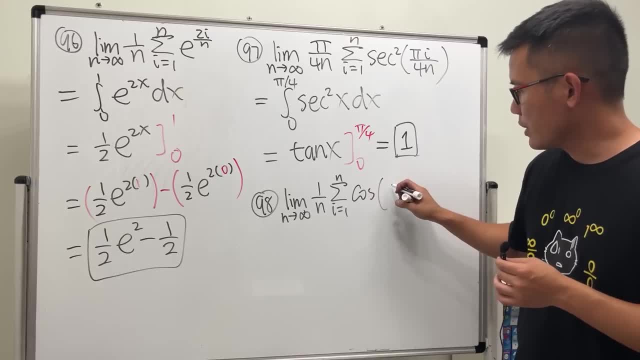 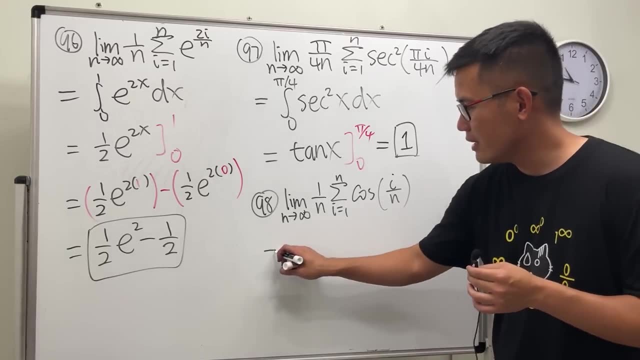 And then we have cosine. This is crazy, It's just i over n. Wow, How do we do this? Well, same idea: Integral 0 to 1, because it's still 1, yeah, 1 over n, 1 over n- match. 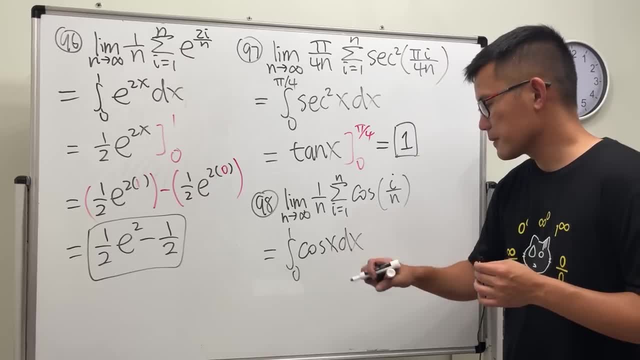 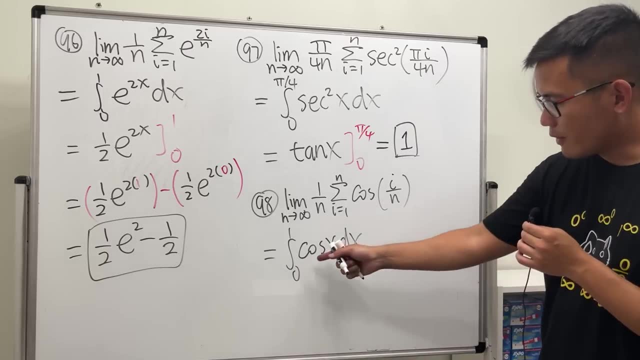 So this is just Cosine x, dx. okay, Yeah, and then let's just go ahead. integrate this. The rule of the fourth. the rule of the fourth function will give us cosine. The answer for that is just sine x. 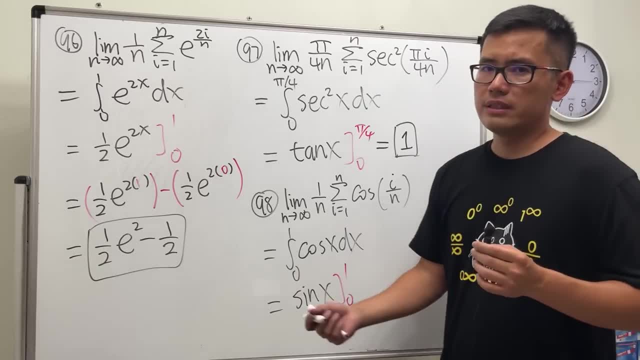 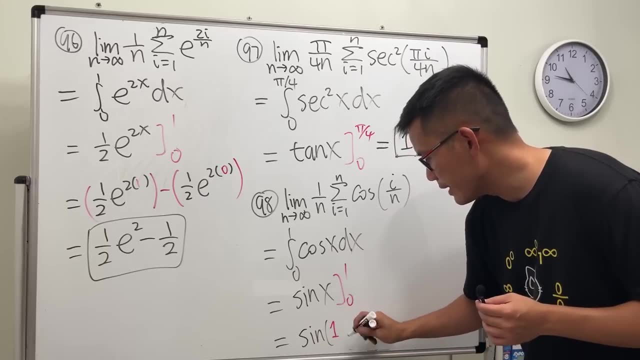 Positive though. Plugging 1, sine of 1, it's a number, it's legit, just leave it. It's not like a special value. you cannot really simplify it, So it's just sine of 1.. Plugging 0, sine of 0 is 0. 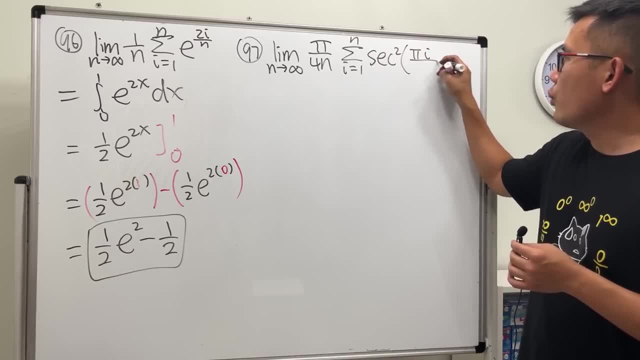 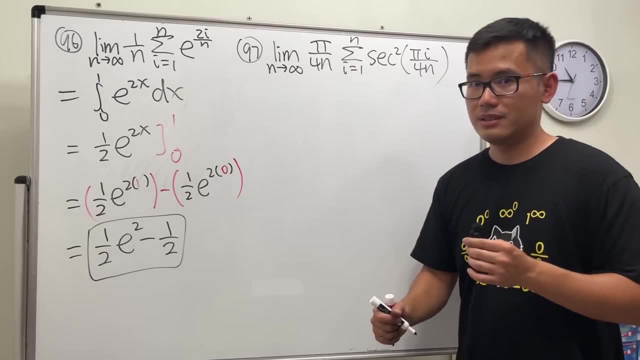 secant square. secant square. pi i over 4 n pi. i over 4 n pi i over 4 n. pi over 4 pi over 4 match pi over 4 pi over 4 match. pi over 4 pi over 4 match. this means we go from 0 to pi over 4. 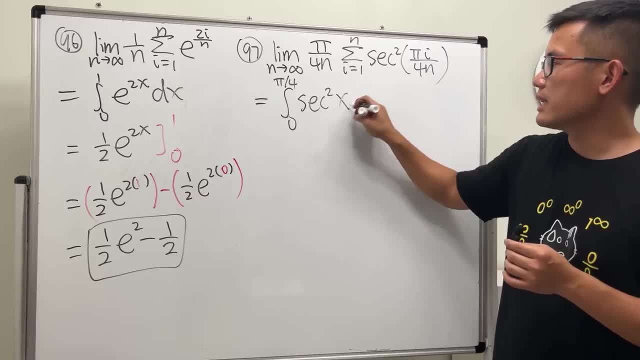 this means we go from 0 to pi over 4. this means we go from 0 to pi over 4 and the input is just what secant and the input is just what secant and the input is just what secant: square x, square x. 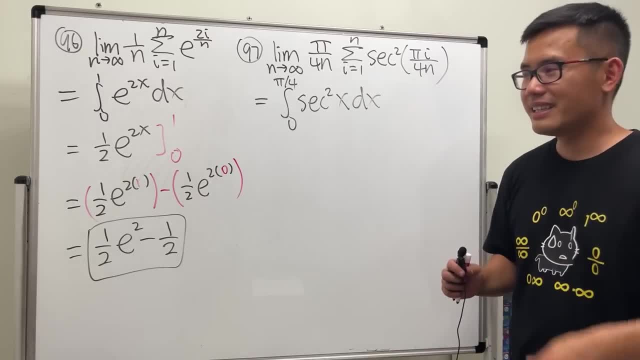 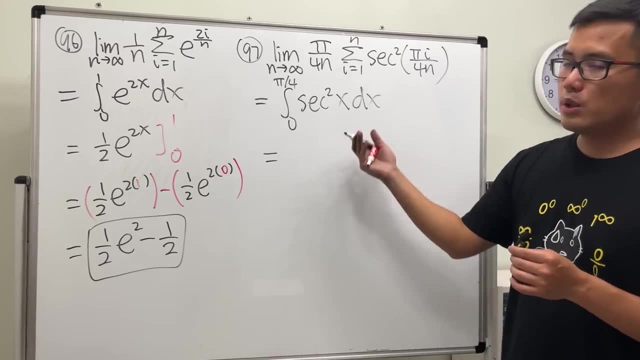 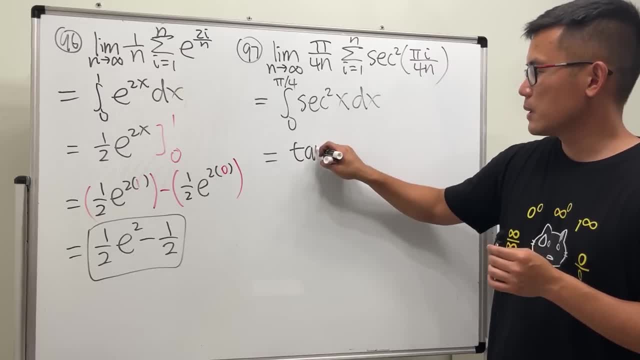 the derivative. what function will give us the derivative? what function will give us secant square, secant square, secant square. the answer is tangent. the answer is tangent. the answer is tangent. so tangent x 0 pi over 4. so tangent x 0 pi over 4. 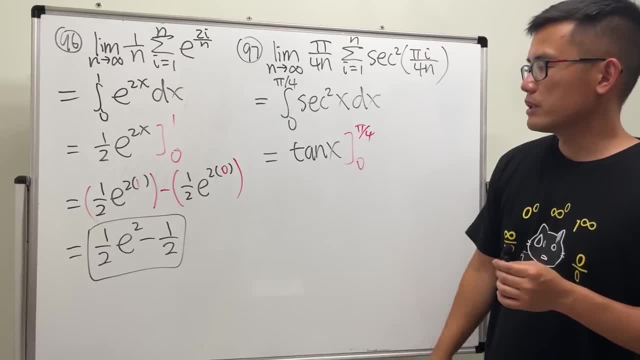 so tangent x 0 pi over 4: plugging power 4. tangent on power 4 is plugging power 4. tangent on power 4 is plugging power 4. tangent on power 4 is 1 plugging 0. tangent of 0 is: 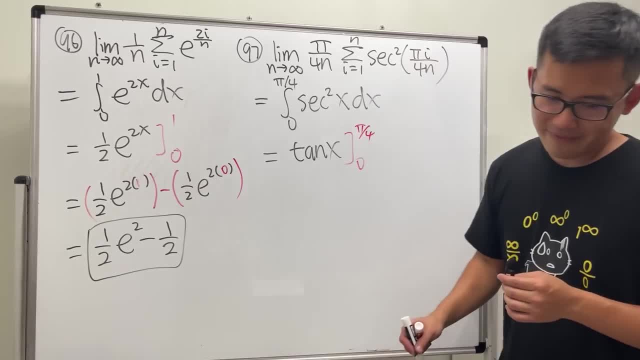 1. plugging 0 tangent of 0 is 1. plugging 0: tangent of 0 is 0. so, all in all, the answer is just 0. so, all in all, the answer is just 0. so, all in all, the answer is just 1. 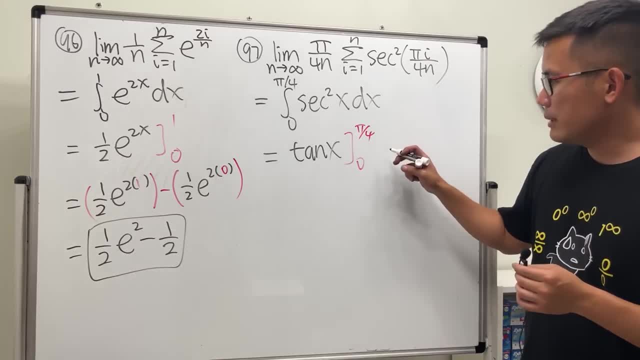 1, 1. so nice, so nice, so nice, yeah. so i'm just going to, yeah, so i'm just going to, yeah, so i'm just going to ready right here, because i want to fit ready right here, because i want to fit ready right here, because i want to fit another question here. 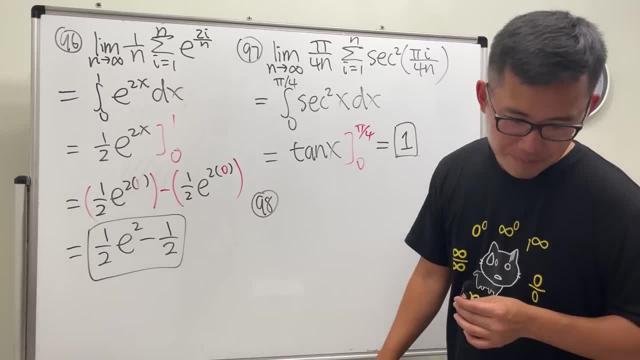 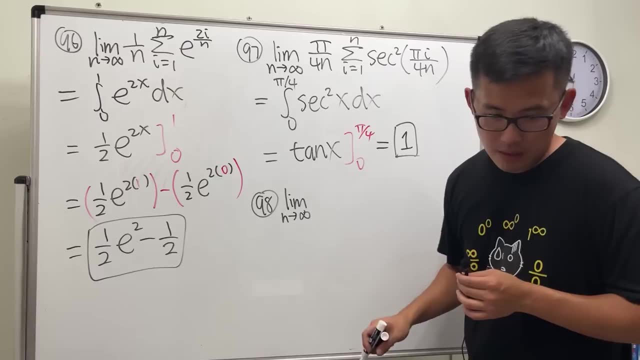 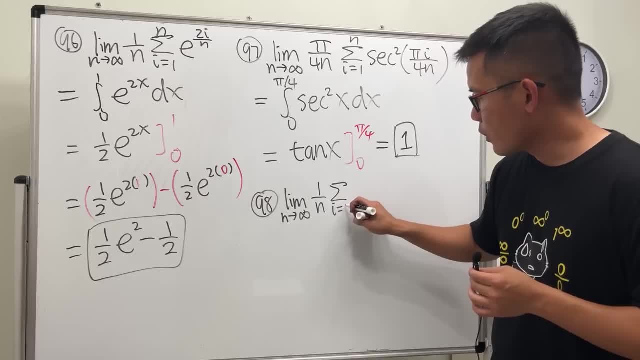 and then we have, and then we have: 1 over n, 1 over n, 1 over n- sigma. i goes from 1 to n sigma. i goes from 1 to n sigma, i goes from 1 to n, and then we have cosine, and then we have cosine. 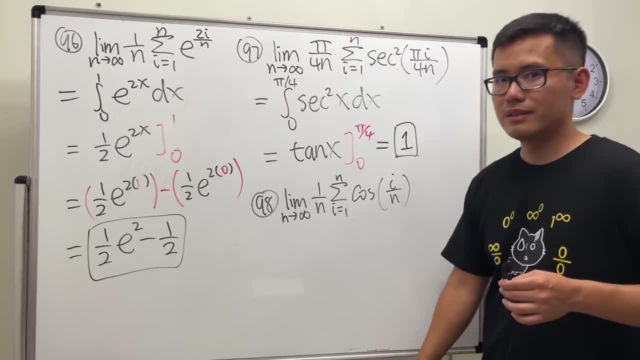 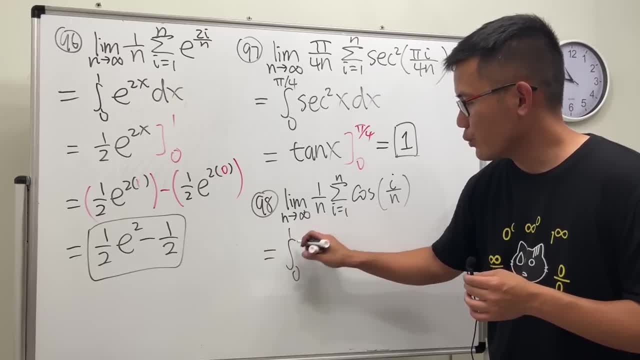 how do we do this? well, same idea. well, same idea. well, same idea. integral 0 to 1, because it's so 1. yeah, integral 0 to 1, because it's so 1, yeah, integral 0 to 1, because it's so 1. yeah, 1 over n, 1 over n. match. so this is just. 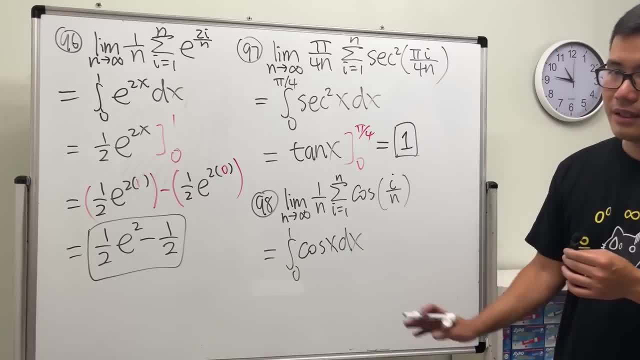 1 over n, 1 over n match. so this is just 1 over n, 1 over n match. so this is just: cosine x dx, cosine x, dx, cosine x dx. okay, okay, okay, yeah, and then let's just go ahead. yeah, and then let's just go ahead. 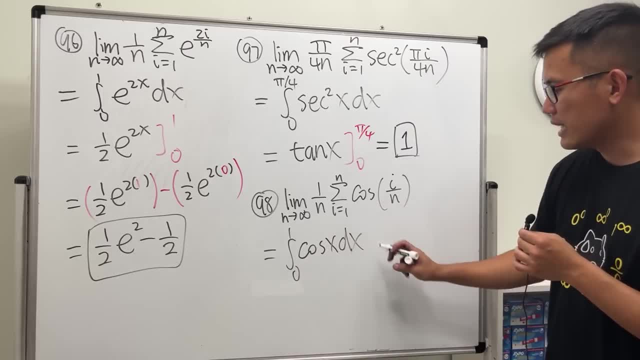 yeah, and then let's just go ahead, integrate this derivative, integrate this derivative, integrate this derivative derivative function will give us cosine. the derivative function will give us cosine. the derivative function will give us cosine the answer for that is just sine answer, for that is just sine answer, for that is just sine x positive though. 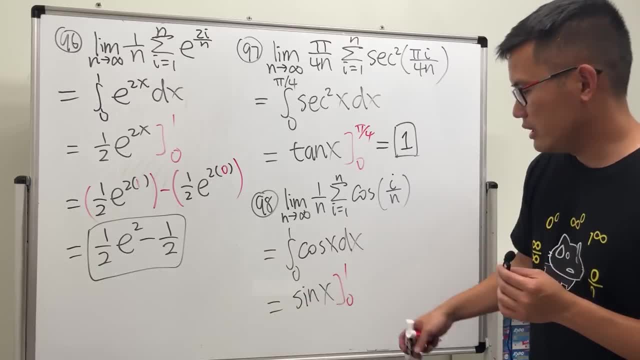 x positive though. x positive though. plugging one sign of one, it's a number. plugging one sign of one, it's a number. plugging one sign of one, it's a number, it's legit, just leave it. it's not like a. it's legit, just leave it. it's not like a. 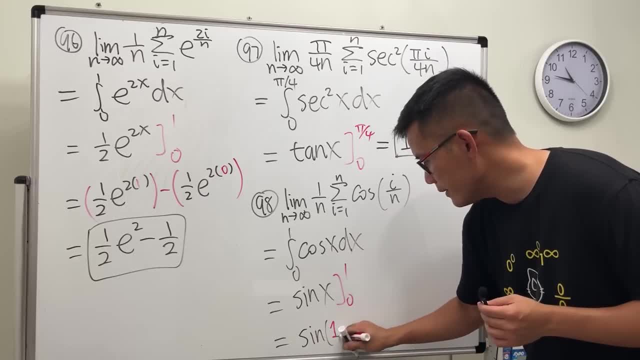 it's legit, just leave it. it's not like a special value. you cannot really special value. you cannot really special value. you cannot really simplify such a sign of one, simplify such a sign of one, simplify such a sign of one. plugging zero sign of zero is zero. so 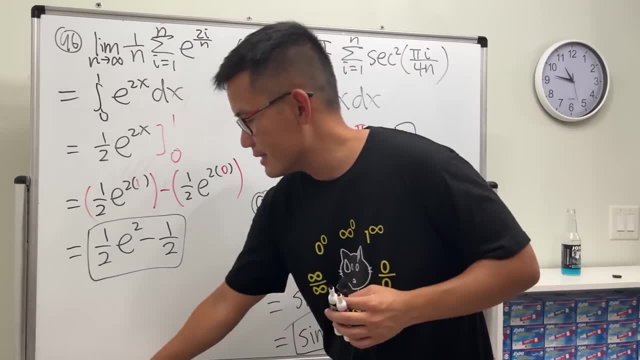 plugging zero sign of zero is zero. so plugging zero sign of zero is zero. so the answer is just sign of one: yeah. so once you know what exactly you yeah. so once you know what exactly you yeah. so once you know what exactly you are looking for, these right here are so. 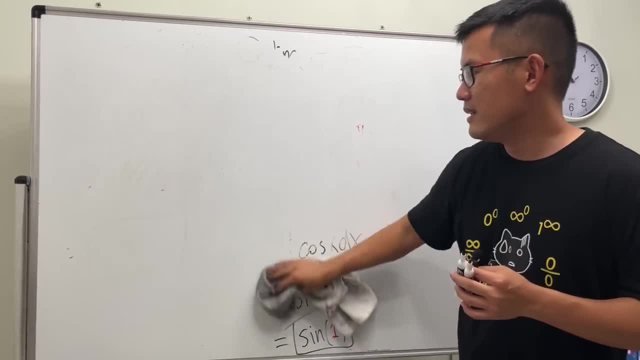 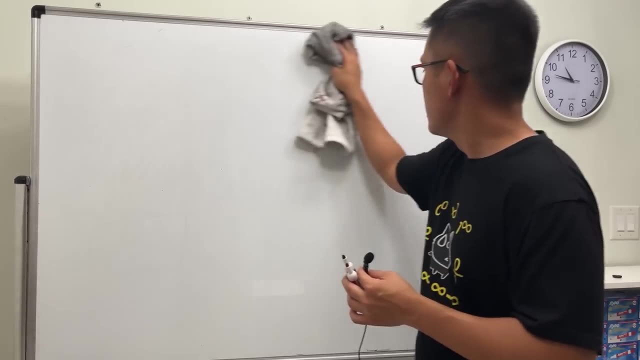 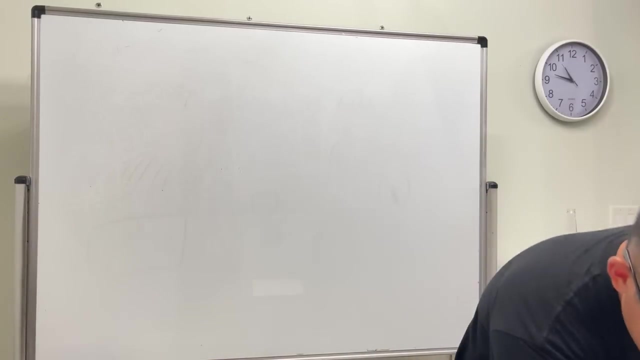 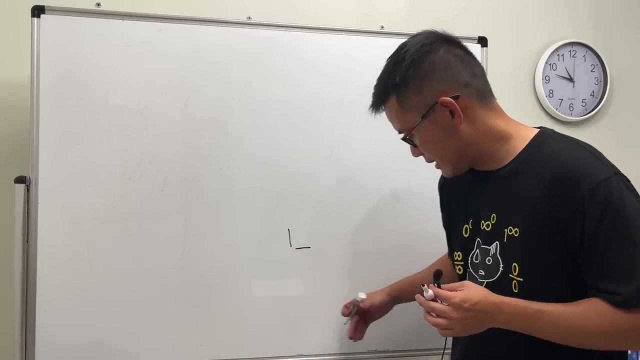 are looking for these right here are. so are looking for these right here. are so beautiful. let me see if i have a better marker. let me see if i have a better marker. let me see if i have a better marker here. maybe ladies and ladies and ladies and jen. 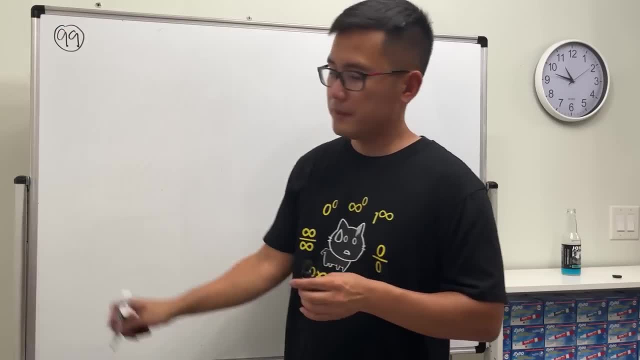 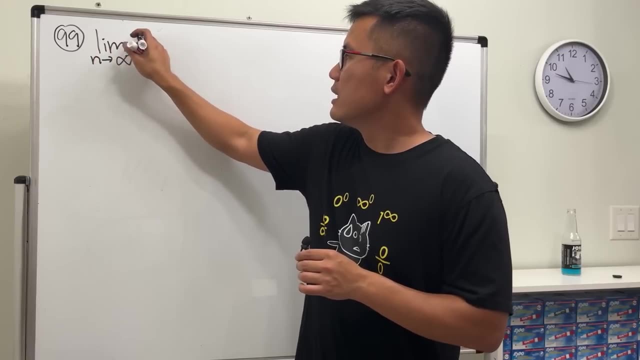 jen jen jen ladies and jen jen ladies and jen jen. number 99: number 99, number 99. all right, all right, all right. limit: this is another expanded version. you limit: this is another expanded version. you limit: this is another expanded version. you guys will see why this is not. 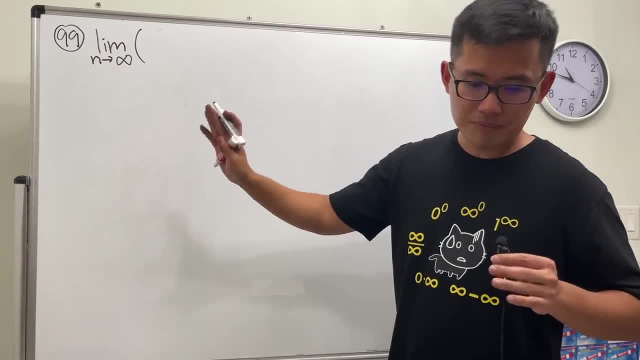 guys will see why this is not. guys will see why this is not. wow, this is number 99 already okay. wow, this is number 99 already okay. wow, this is number 99 already okay. focus, focus, focus. n n n over n square plus one plus over n square plus one plus. 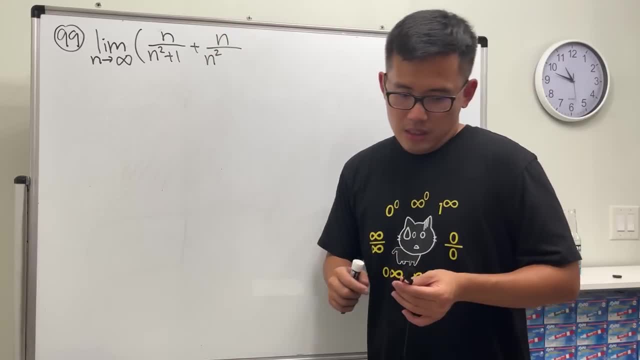 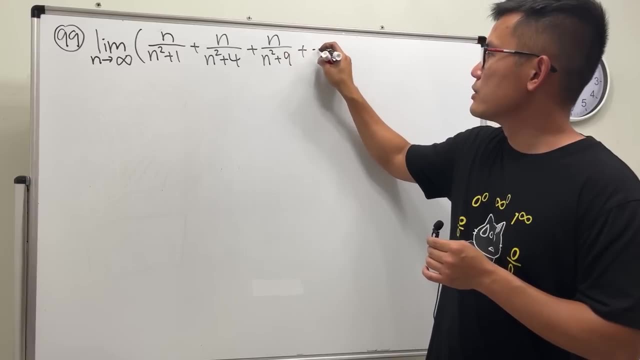 over n square plus one plus n over n square n over n square plus n over n square plus four, four, four plus n over n square plus plus n over n square plus plus n over n square plus nine, so on, so on, so on, up to nine, so on, so on, so on, up to. 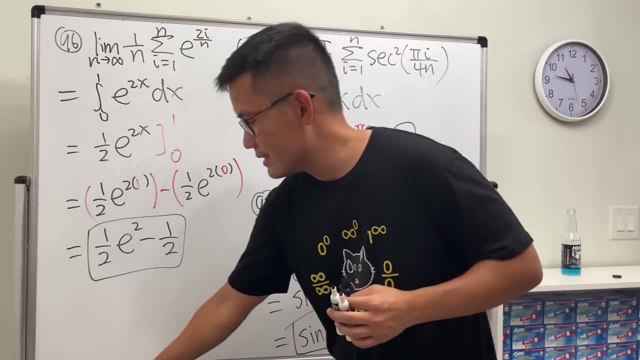 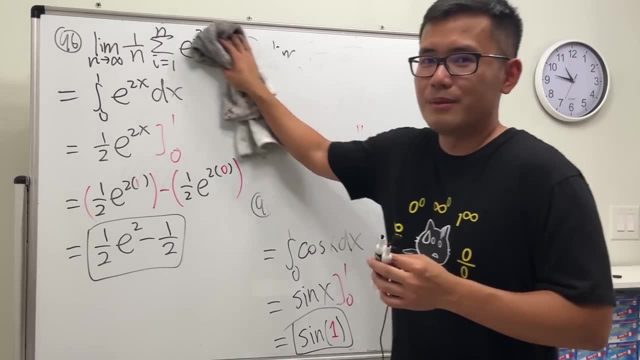 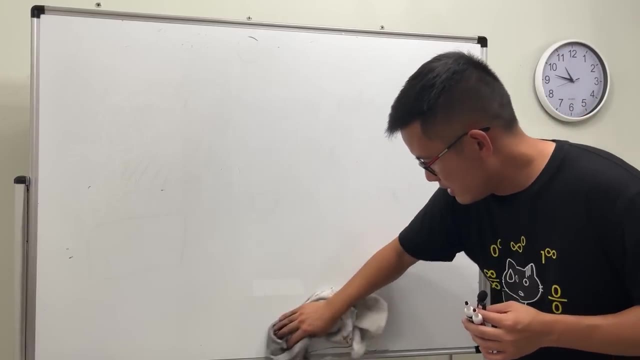 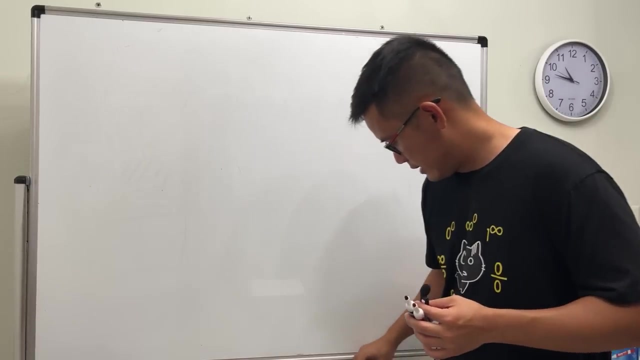 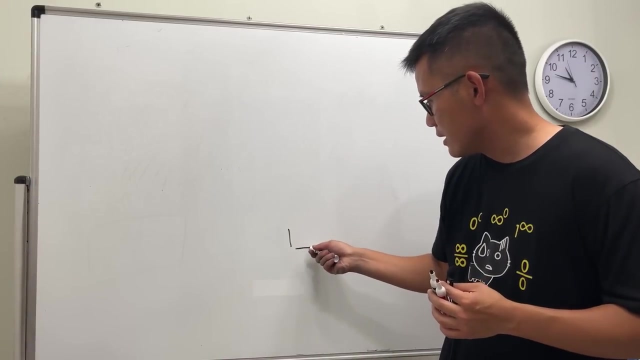 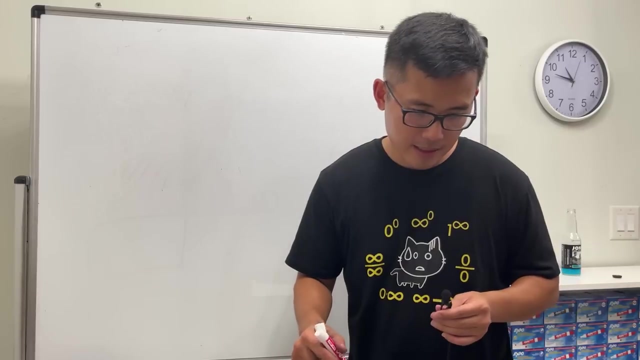 So the answer is just sine of 1.. It's a number, Yeah. So once you know exactly what you are looking for, these right here are so beautiful. Let me see if I have a better marker here. Maybe, Ladies and gentlemen, number 99.. 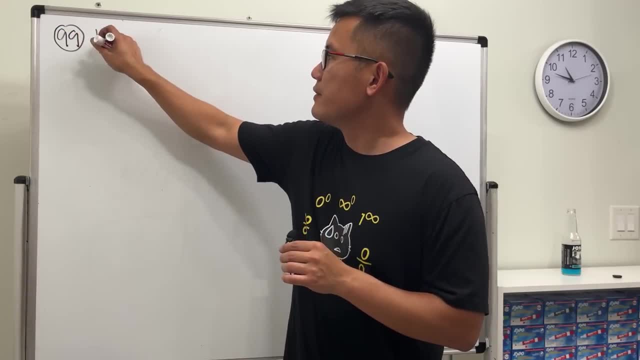 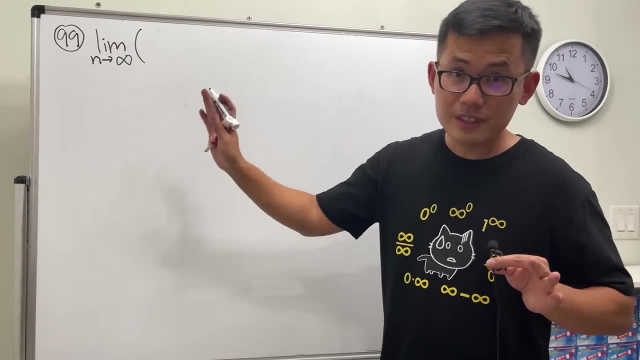 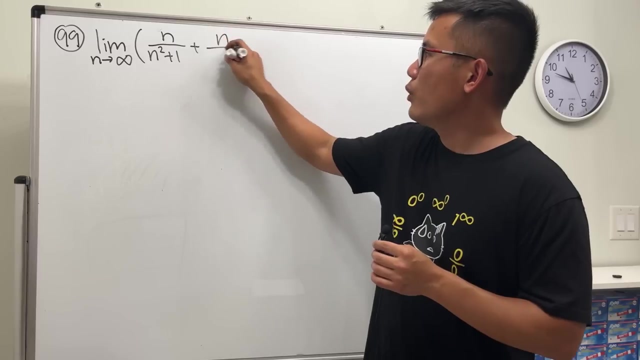 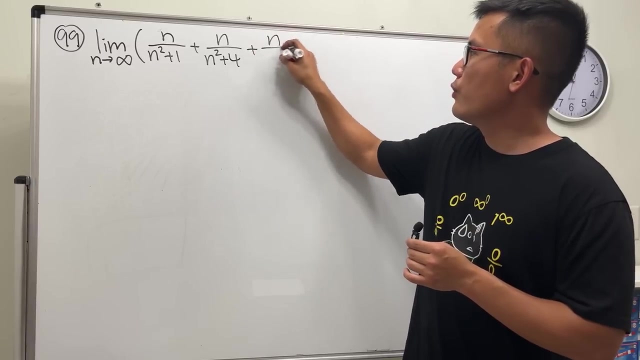 Alright Limit. This is another expanded version. You guys will see why this is not. Wow, this is number 99 already. Okay, Focus: N over N squared plus 1. Plus N over N squared plus 4.. Plus N over N squared plus 9.. 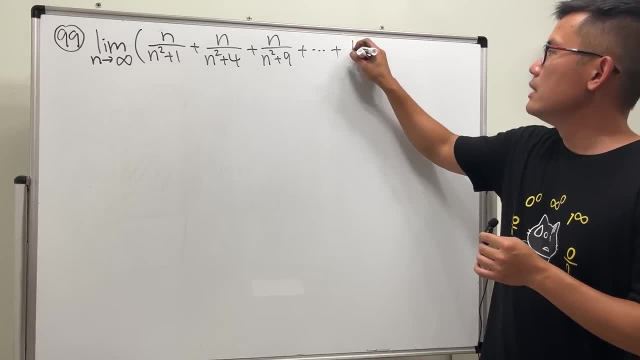 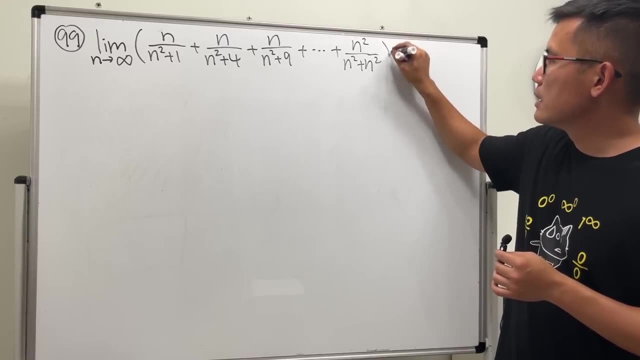 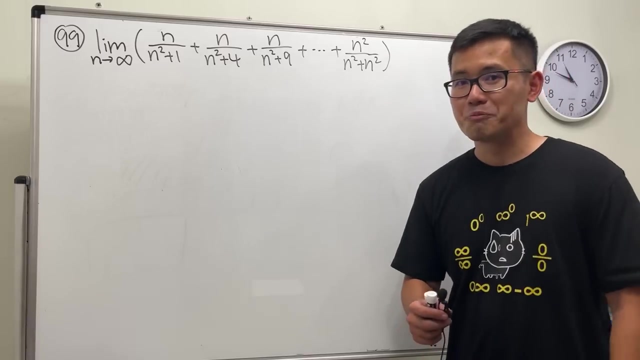 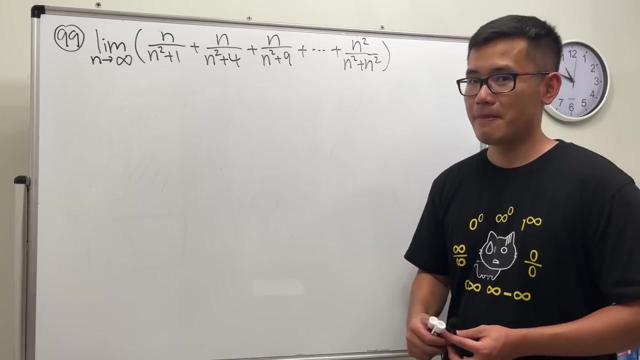 So on, so on, so on. Up to Wow, N squared over N squared plus N squared. Oh my god, Where is the over N part? huh, Where is it? Pause the video. Give this a try first Done. 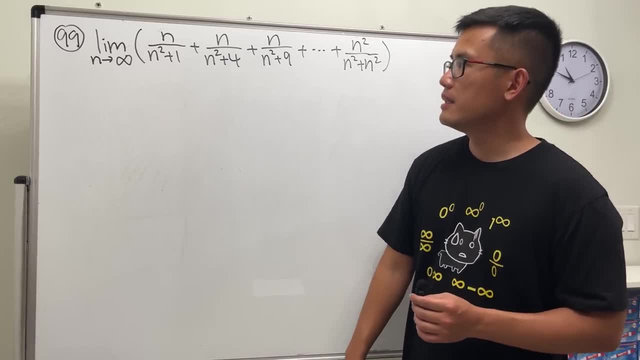 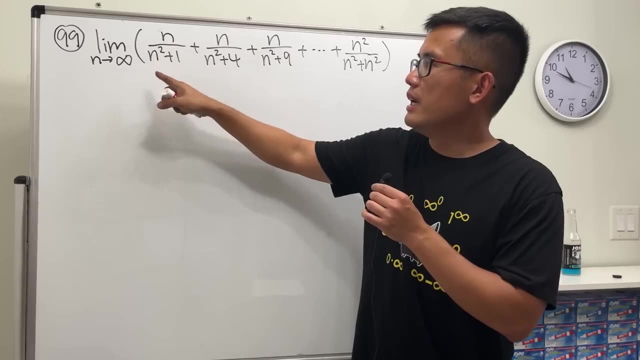 By the way, let's do this. Huh, When you see this kind of question, do not just do the following and say: Put the infinity here and here and say, hey, the degree right here is bigger than that. So the answer is 0 for the first one. 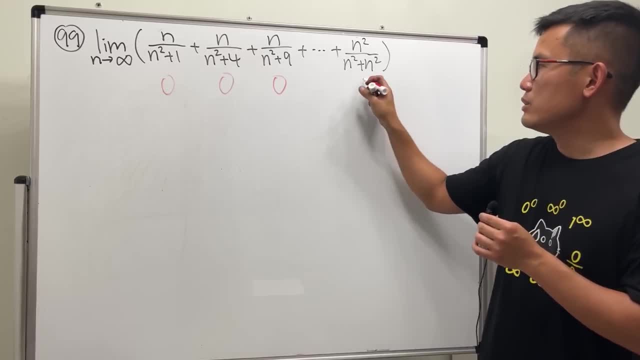 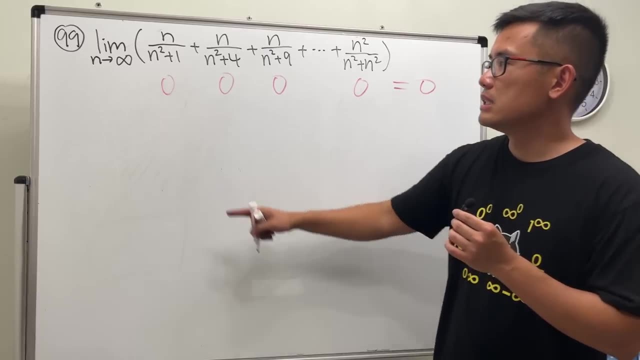 And the next one is 0.. 0 and then just 0. So we're just adding a bunch of 0s, huh, So the answer should just be 0?? No, Because the limit is 0.. Think about this as 0+. 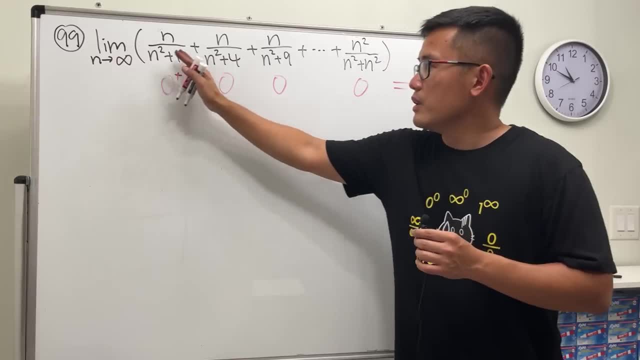 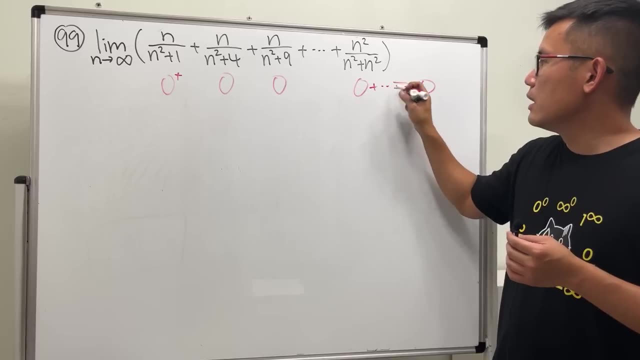 And another thing is that, as N goes to infinity, we have- how many terms You see the plus dot, dot, dot, and this has N. We actually have infinitely many of this kind of things. So this is almost like saying 0 times infinity in determinant form. 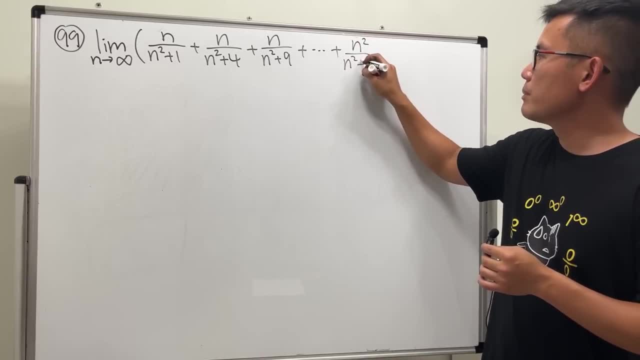 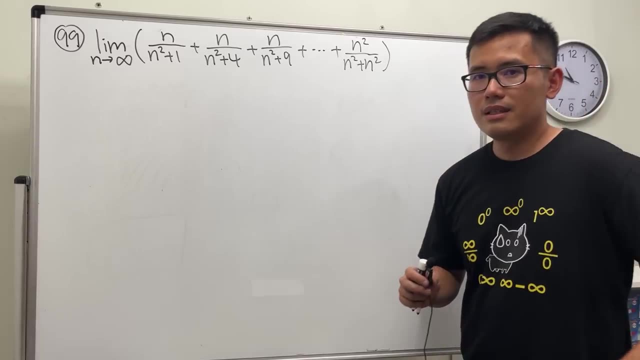 nine, so on, so on, so on, up to wow, wow, wow, n square over n square plus n n square over n square plus n n square over n square plus n square. oh, my god, where is the open end part? huh, where is? where is the open end part? huh, where is? 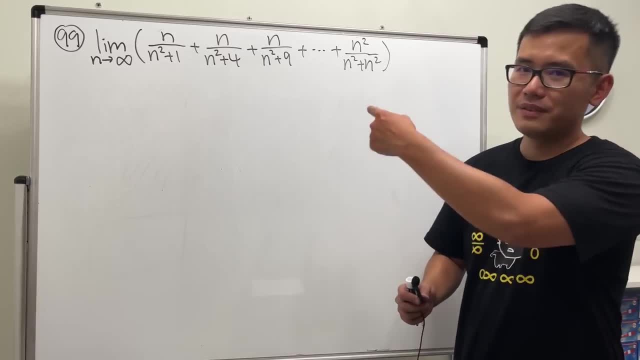 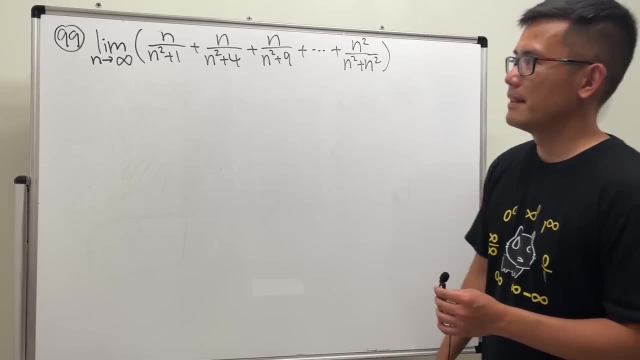 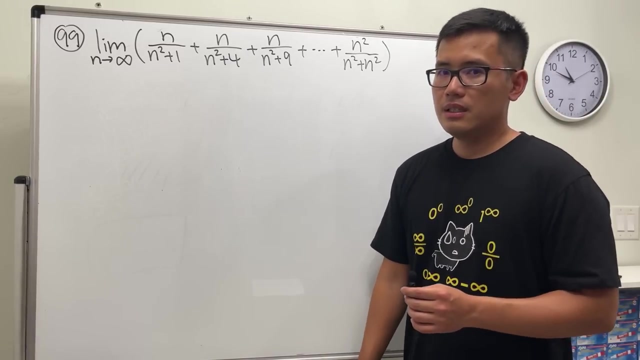 where is the open end part? huh, where is it? pause the video. give this to try first. pause the video. give this to try first. pause the video. give this to try first. done, done, done, by the way, let's do this. by the way, let's do this. 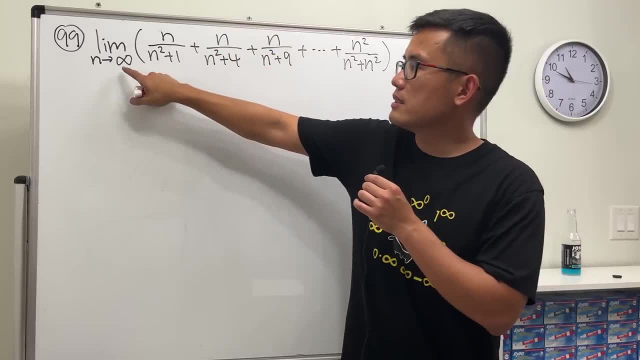 by the way, let's do this when you see this kind of question. do not, when you see this kind of question, do not, when you see this kind of question, do not just do the following and say just do the following. and say just do the following. and say put the infinity here and here. and say 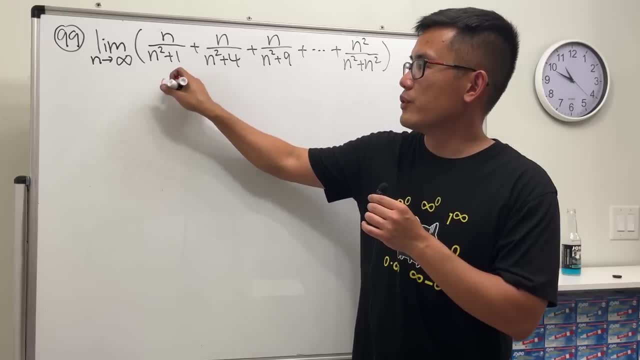 put the infinity here and here and say: put the infinity here and here and say: hey, the degree right here is bigger than hey, the degree right here is bigger than hey, the degree right here is bigger than that. so the answer is zero for the that. so the answer is zero for the. 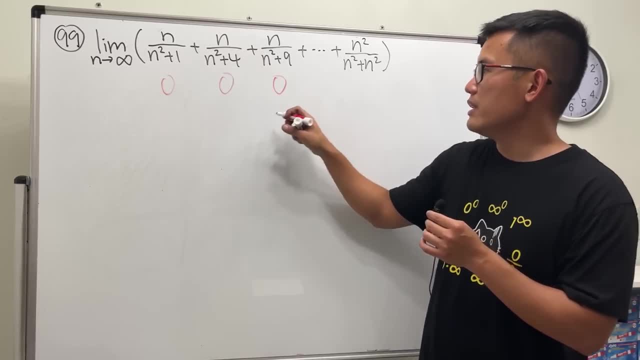 that. so the answer is zero for the first one, and then the next one is zero. first one, and then the next one is zero. first one, and then the next one is zero. likewise zero, and then just zero. so, likewise zero, so, likewise zero. so we're just adding a bunch of zeros, huh. 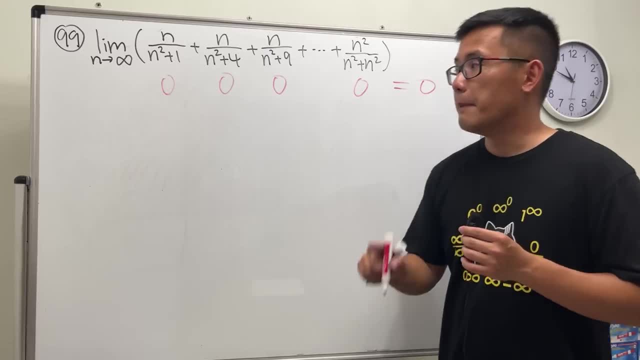 we're just adding a bunch of zeros, huh, we're just adding a bunch of zeros, huh. so the answer should just be zero. so the answer should just be zero. so the answer should just be zero. no, no, no, because, because, because the limit is zero, the limit is zero. 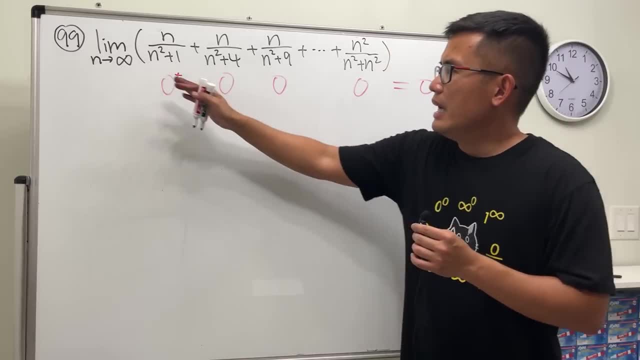 the limit is zero. think about this as zero plus, and think about this as zero plus, and think about this as zero plus, and another thing is that. another thing is that. another thing is that, as n goes to infinity, we have how many. as n goes to infinity, we have how many. 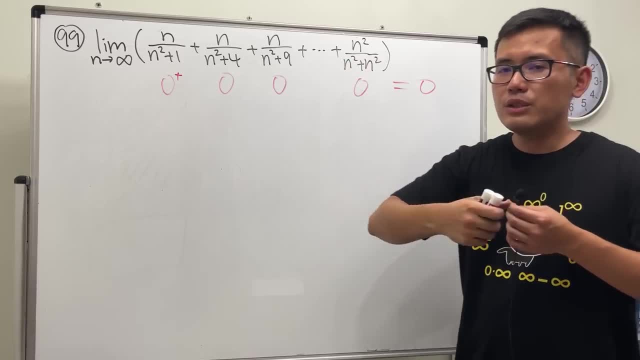 as n goes to infinity. we have how many terms, terms, terms. you see the plus dot dot dot, and this, you see the plus dot dot dot, and this, you see the plus dot dot dot, and this has n, has, n, has n. we actually have infinitely many of this. 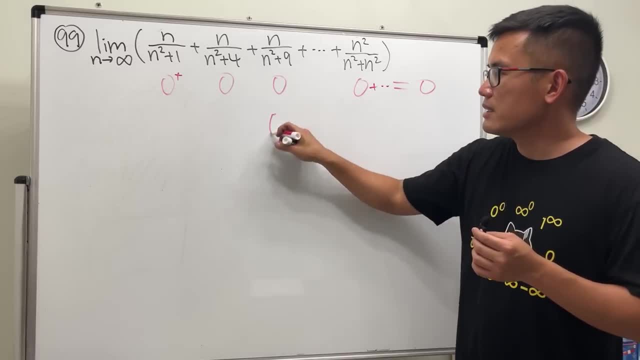 we actually have infinitely many of this. we actually have infinitely many of this kind of things, kind of things, kind of things. so this is almost the same zero times. so this is almost the same zero times. so this is almost the same zero times: infinity in the form. so 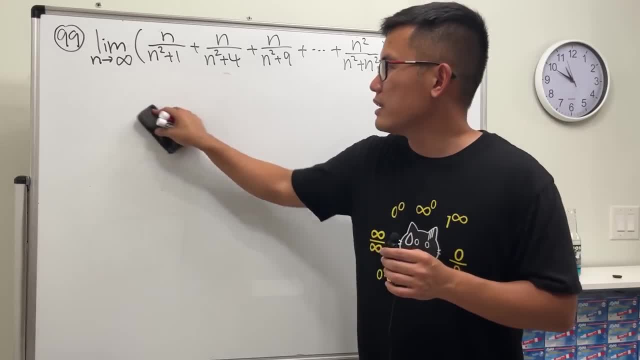 infinity in the form. so infinity in the form. so cannot say, cannot say, cannot say any answer, any answer, any answer unless we do more work, unless we do more work, unless we do more work. it's a different kind of indeterminate. it's a different kind of indeterminate. 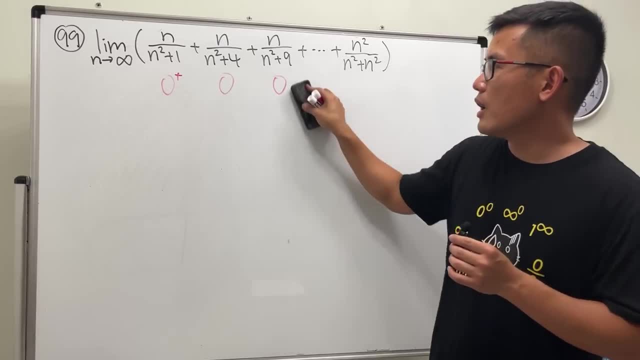 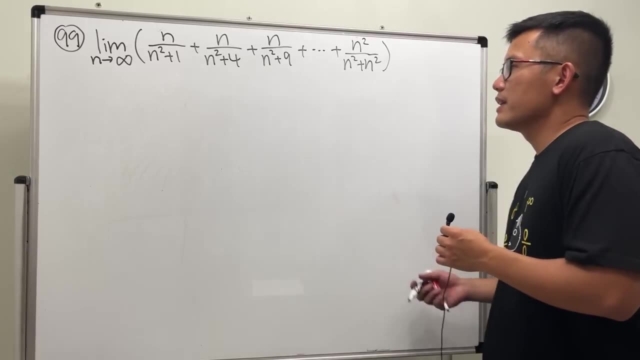 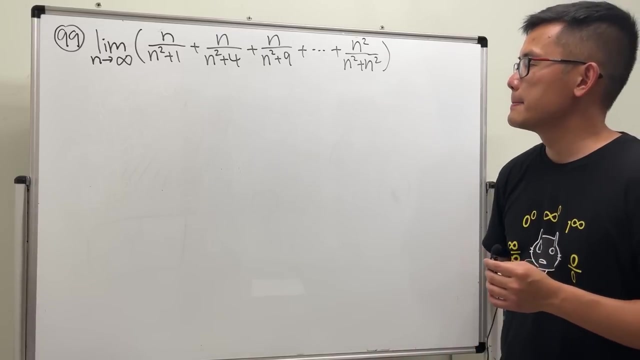 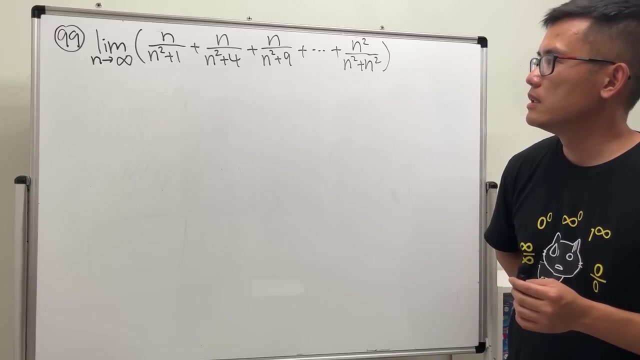 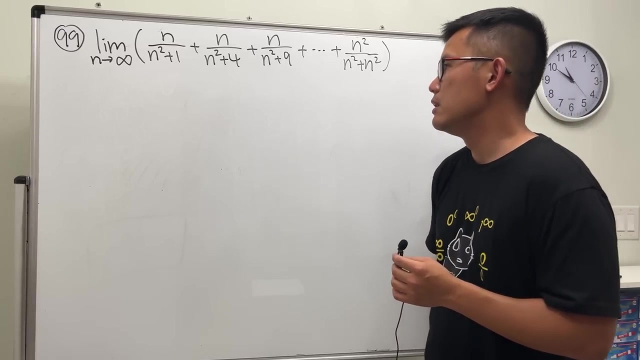 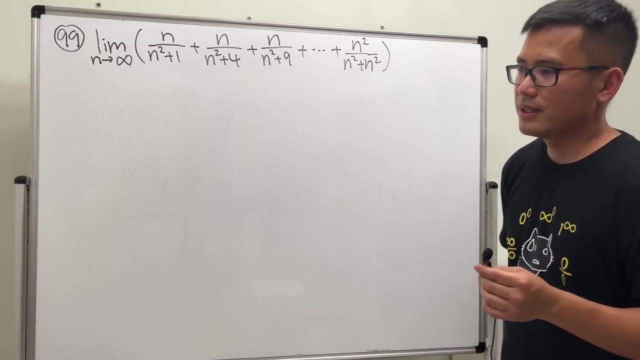 So cannot say Any answer unless we do more work. It's a different kind of indeterminate form. Okay, so how exactly do we do it, though? Again, we want to see the sum number over N part. Let's see. I know the answer, but like I just have to think about how to explain it so that I don't give it away right away. 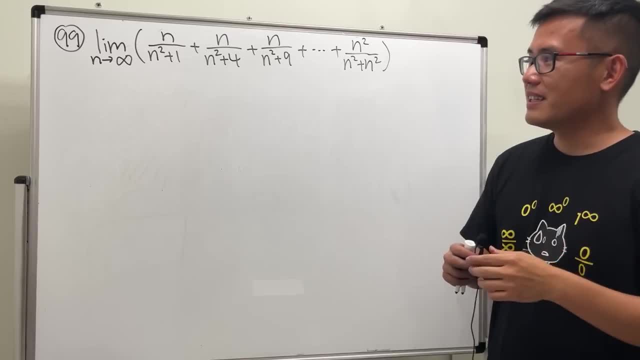 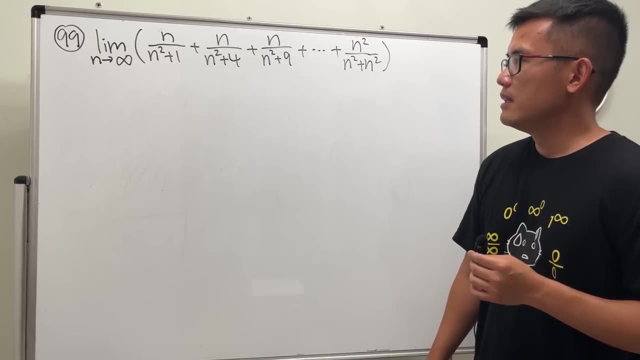 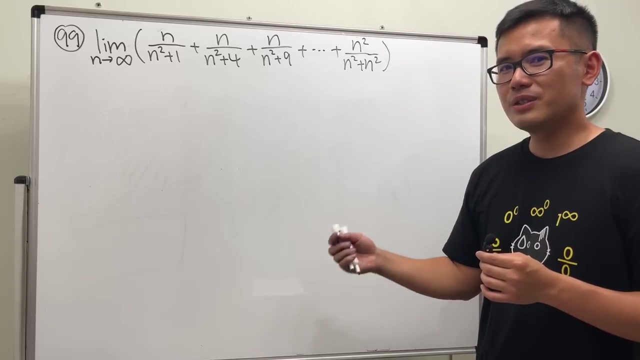 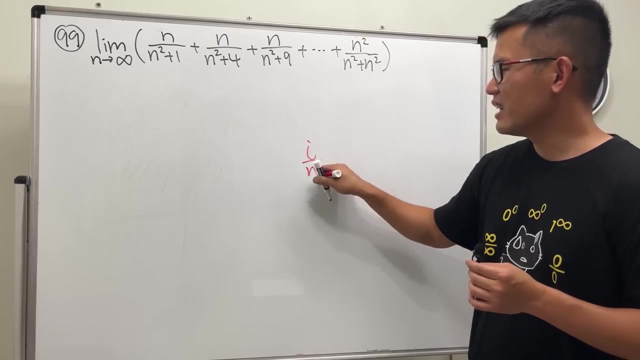 Number 99 is tough, It's not easy. All right, 1,, 4,, 9.. Hey, they look suspicious, Aren't they just a 1 square, 2 square, 3 square and so on. And remember, we want to have, like I, over N huh. 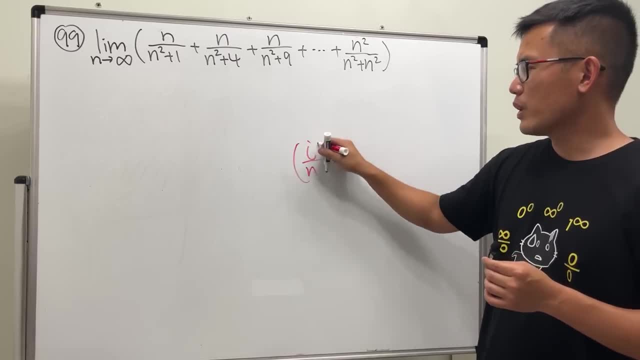 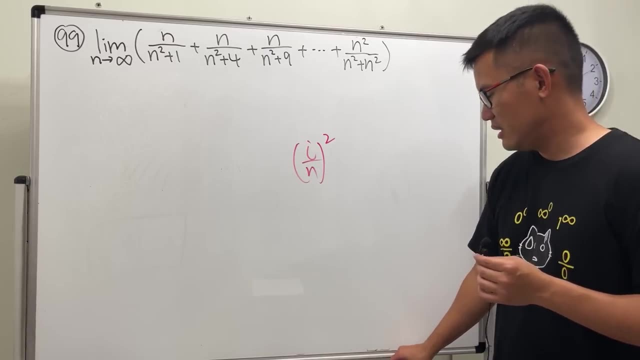 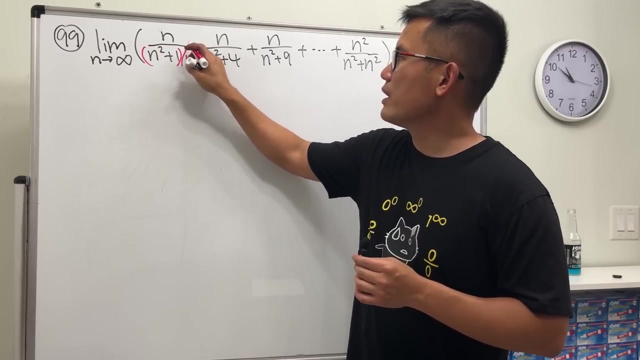 And then, because it's a 1 square, 2 square, 3 square, so maybe we want to produce I over N square somehow. So let's do the following Right here: let's divide this by N square And, of course, do the same on the top. 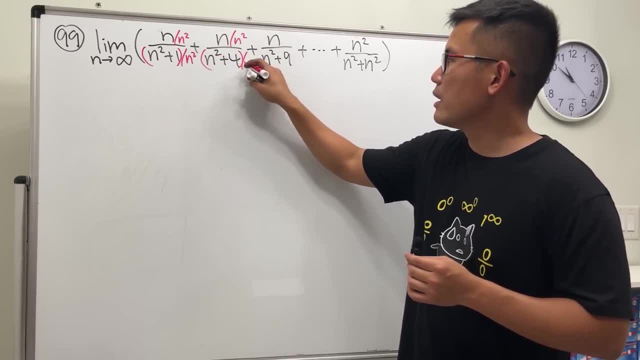 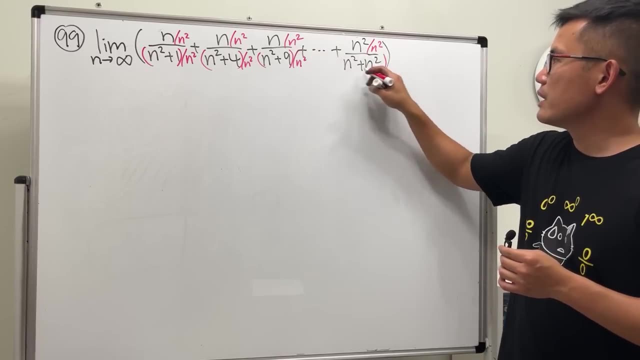 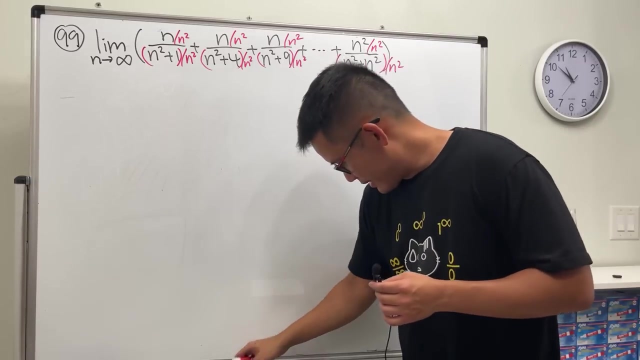 Divide this by N square and do the same right here, And divide this by N square, do the same, and then divide this by N square, and then do the same. What good does this do? Let's see. Okay, now I have to look for a marker that works. 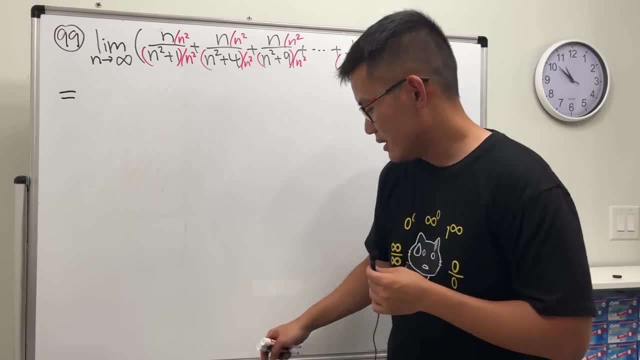 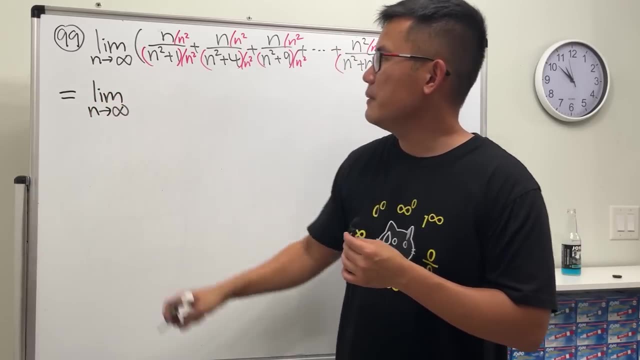 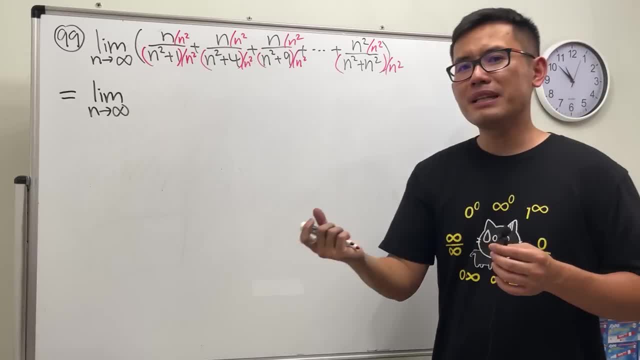 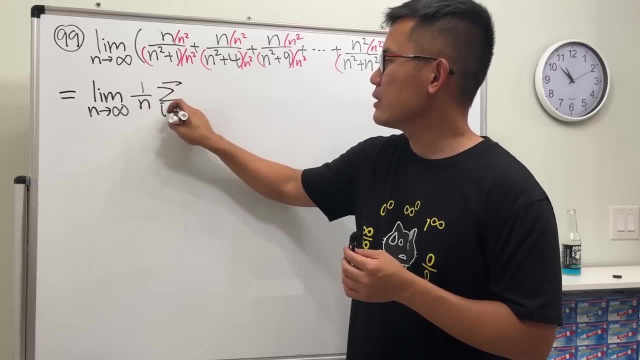 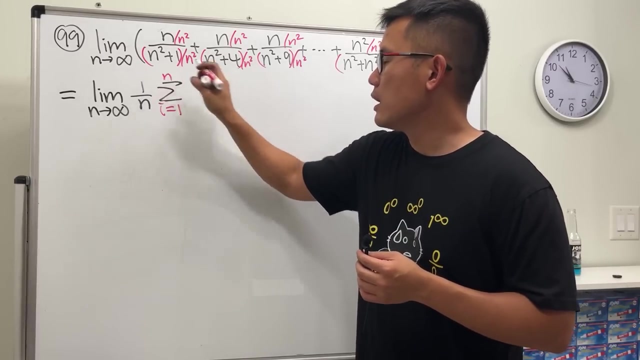 If we have N over N, square on the top, everybody has a 1 over N. now, Perfect, Let's factor that out, Put it here, And then sum. I goes from 1 to N. All right, And then let's see: 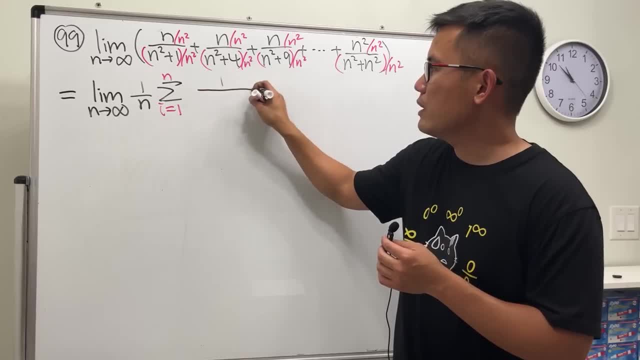 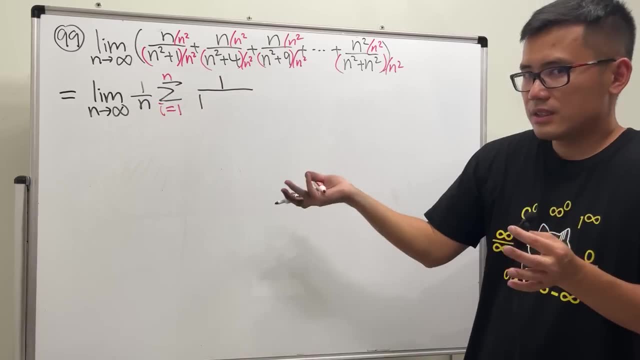 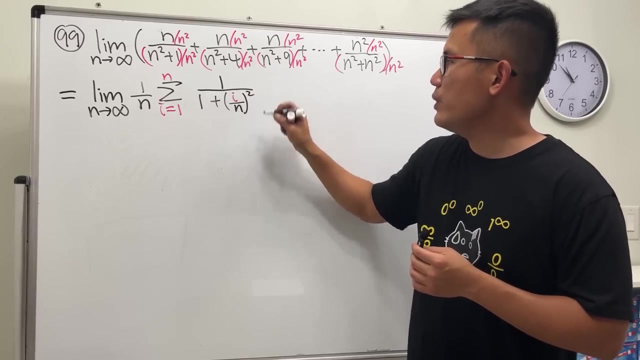 Now, because I put that over there already. so we have a 1 on the top and over N, So this over that is just 1, and 1 square over n square, as we said earlier. that's exactly what we want. huh, that's plus parentheses. i over n- n square. this is 2 square over n square. 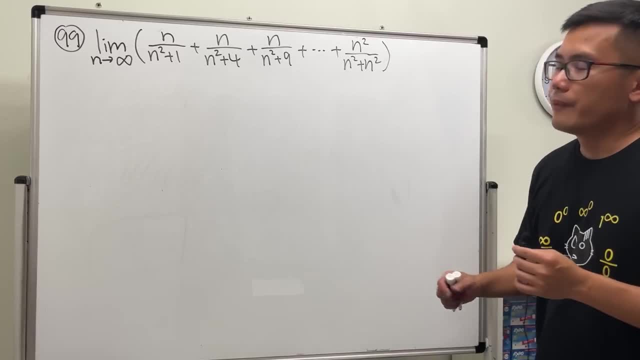 it's a different kind of indeterminate form: form form. okay. so how exactly do we do it though? okay, so how exactly do we do it though? okay, so how exactly do we do it? though? again, we want to see the sum number. again, we want to see the sum number. 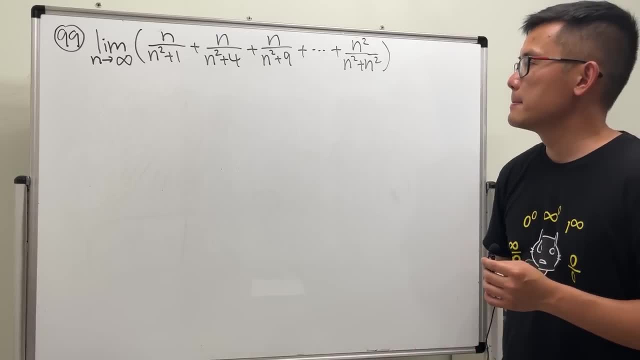 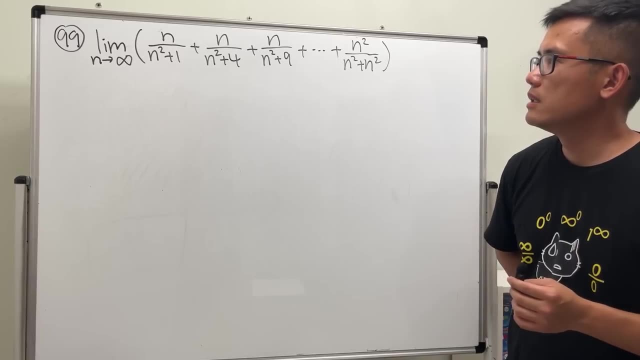 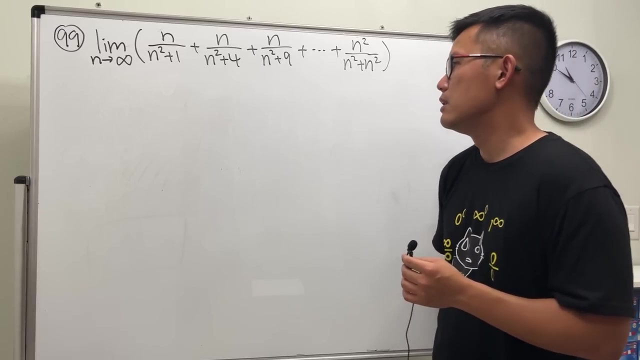 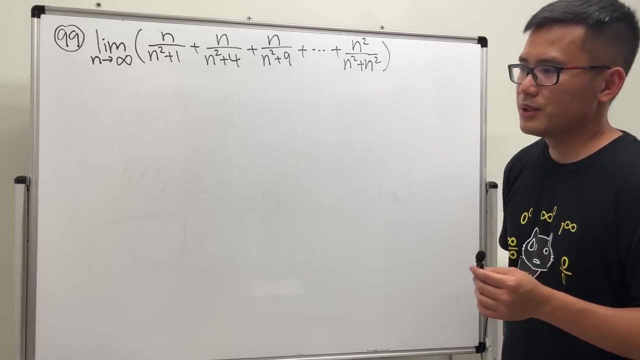 again, we want to see the sum number over m part. let's see. i know the answer, but, like i just have, i know the answer, but like i just have, i know the answer, but like i just have to think about how to explain it so that, to think about how to explain it so that. 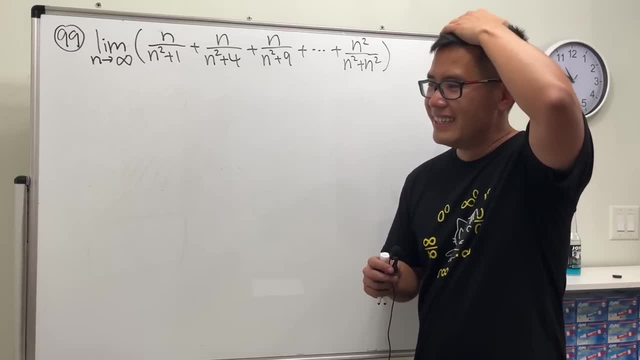 to think about how to explain it, so that i don't give it away right away. i don't give it away right away, i don't give it away right away. number 99 is tough, it's not a, it's not. number 99 is tough, it's not a, it's not. 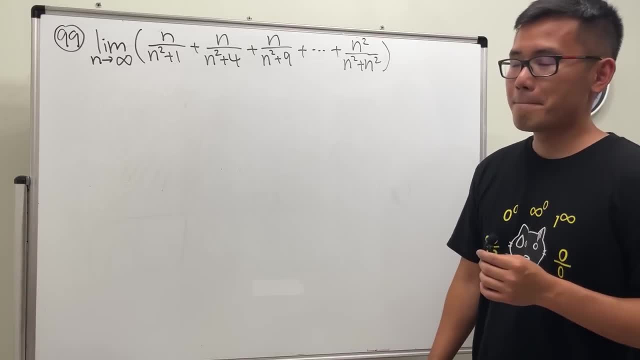 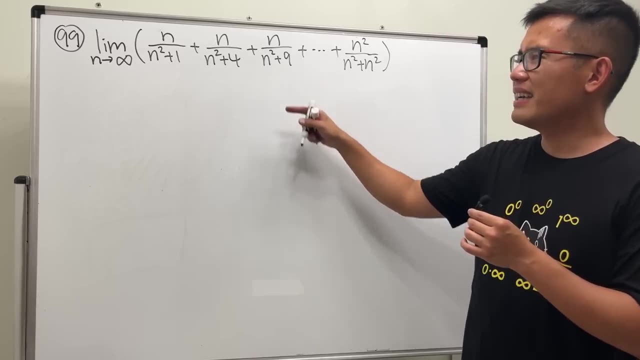 number 99 is tough. it's not a, it's not easy, easy, easy, all right. one, four, nine. hey, they look suspicious. one, four, nine. hey, they look suspicious. one, four, nine. hey, they look suspicious. aren't they just a one square two? aren't they just a one square two? 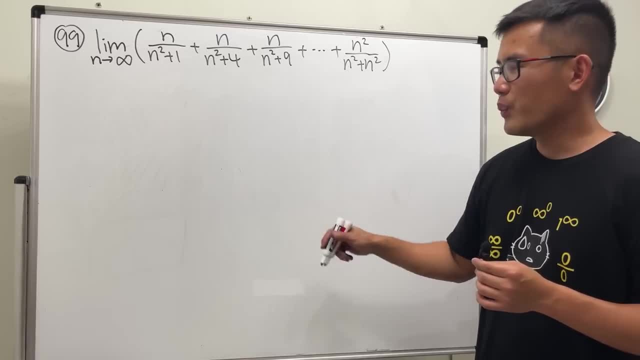 aren't they just a one square, two squares, three squares and so on, squares, three squares and so on, squares, three squares and so on. and remember, we want to have like i over, and remember, we want to have like i over, and remember, we want to have like i over, n huh. 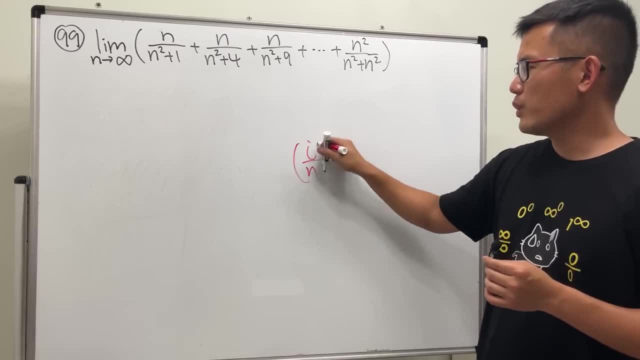 n huh, n huh, and then, because it's a one, square two, and then, because it's a one, square two, and then, because it's a one, square two, square, three, square, so maybe we want to square three, square, three, square, so maybe we want to square three, square, three, square, so maybe we want to produce. 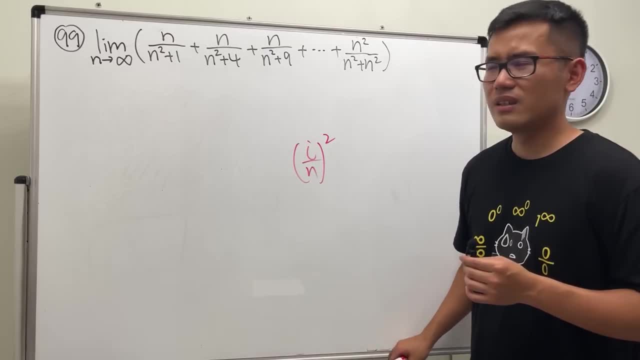 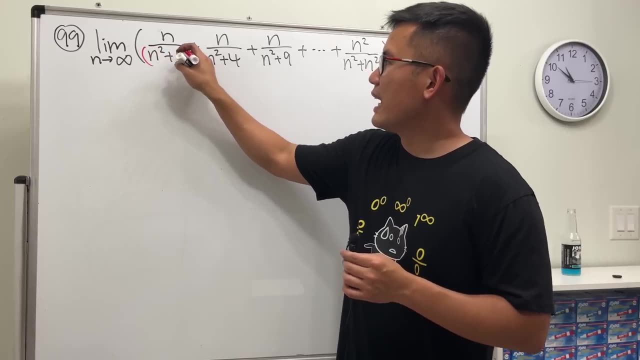 produce, produce, i offer, i offer, i offer, and square somehow, and square somehow, and square somehow. so, so, so, let's do, let's do, let's do the following: the following: the following, right here, right here, right here, let's divide this by. let's divide this by. 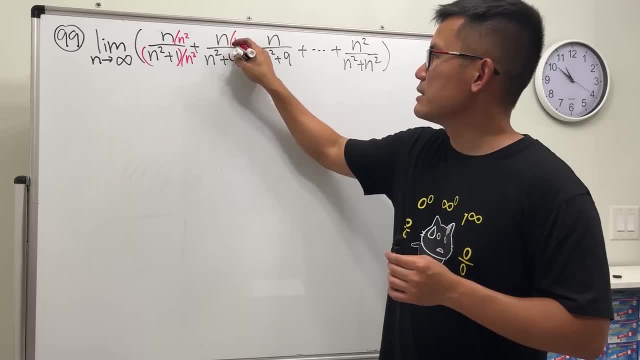 let's divide this by n square and, of course, do the same on n square, and, of course, do the same on n square and, of course, do the same on the top, the top, the top. divide this by n square, divide this by n square. divide this by n square and do the same right here. 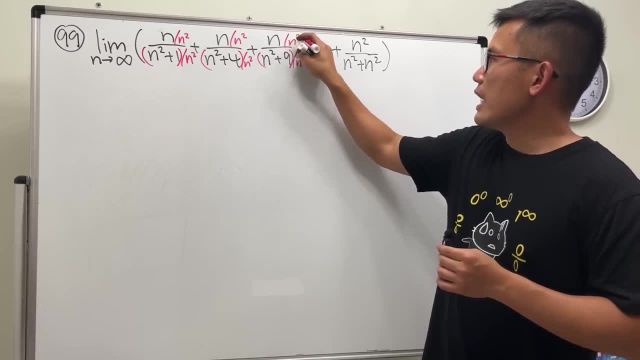 and do the same right here and do the same right here, and divide this by n square and divide this by n square and divide this by n square. do the same and then divide this by n. do the same and then divide this by n. do the same and then divide this by n square. 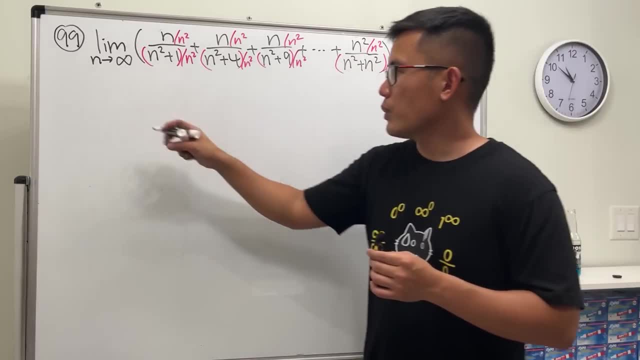 square, square, and then do the same, and then do the same, and then do the same. what good does this do? that's z. what good does this do? that's z. what good does this do? that's z. okay, now i have to look for a marker. okay, now i have to look for a marker. 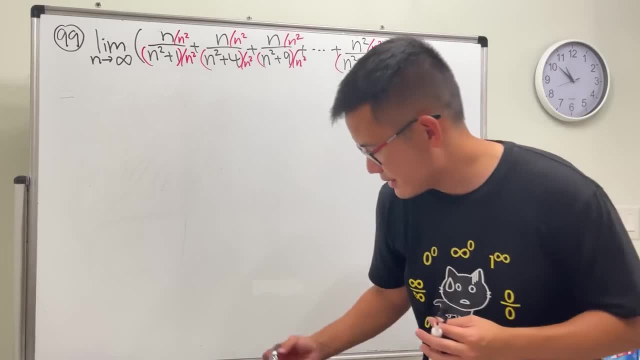 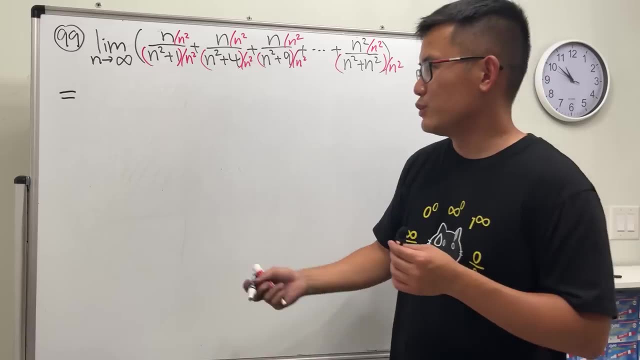 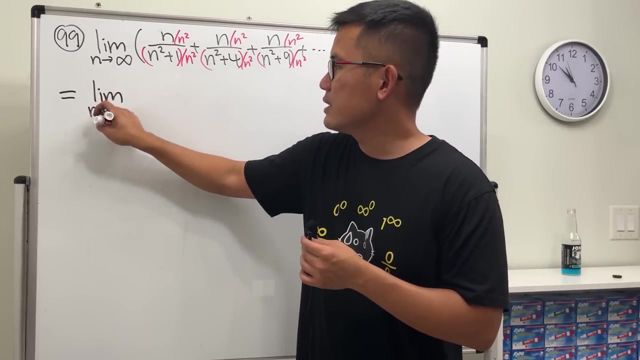 okay, now i have to look for a marker that works. this is the one that i let it rest. this is the one that i let it rest. this is the one that i let it rest earlier. all right, here, we have the limit as n. all right, here, we have the limit as n. 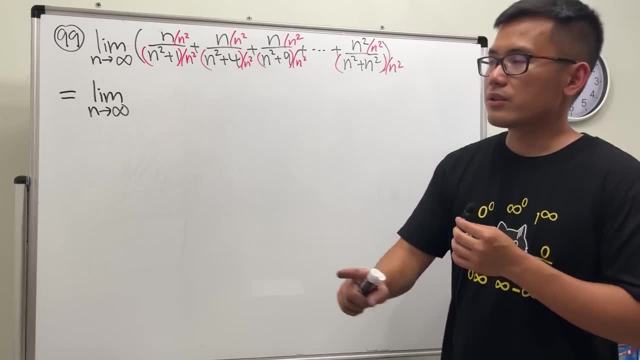 all right, here we have the limit as n goes to, goes to, goes to infinity. check this out if we have infinity. check this out if we have infinity. check this out if we have n over n square on the top, everybody has n over n square on the top, everybody has. 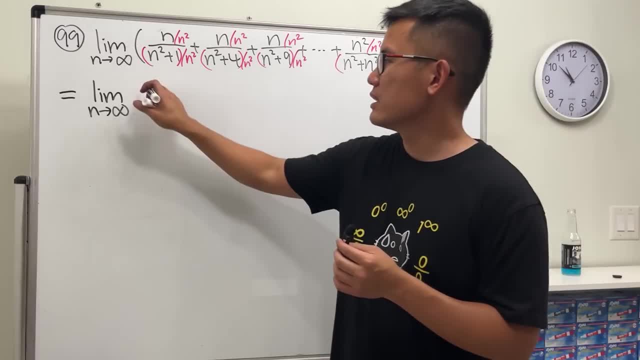 n over n, square on the top, everybody has that. one over n. now. that one over n. now. that one over n, now perfect, let's factor that out, put it here. perfect, let's factor that out, put it here. perfect, let's factor that out, put it here. and then sum. i goes from one to 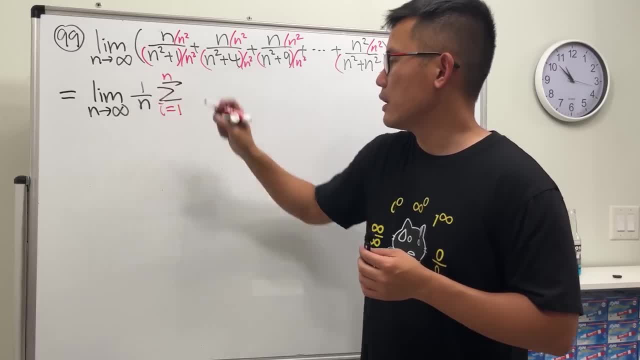 and then sum- i goes from one to, and then sum- i goes from one to n. all right. and then let's see now, because all right. and then let's see now, because all right. and then let's see now, because i put that over there already, so we have. 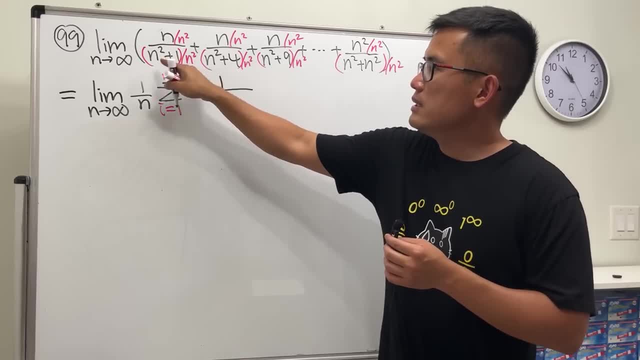 i put that over there already, so we have. i put that over there already. so we have a one on the top and over, a one on the top and over, a one on the top and over this. over, that is just one and one. this over, that is just one and one. 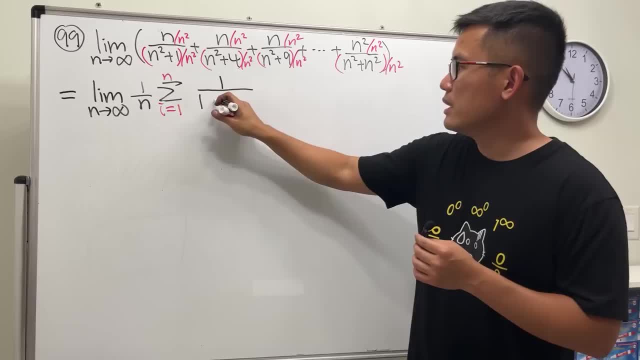 this over. that is just one and one. square over n square, as we said earlier. square over n square, as we said earlier. square over n square, as we said earlier. that's exactly what we want. huh, that's exactly what we want. huh, that's exactly what we want. huh, that's plus parentheses. 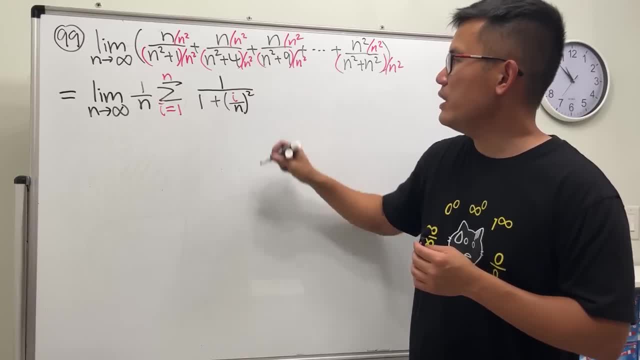 that's plus parentheses. that's plus parentheses. i over n and square. i over n and square. i over n and square. this is two square over n square. this is two square over n square. this is two square over n square. this is three square over n square, so on. 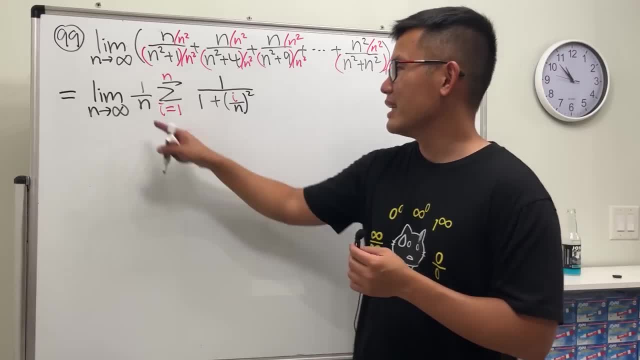 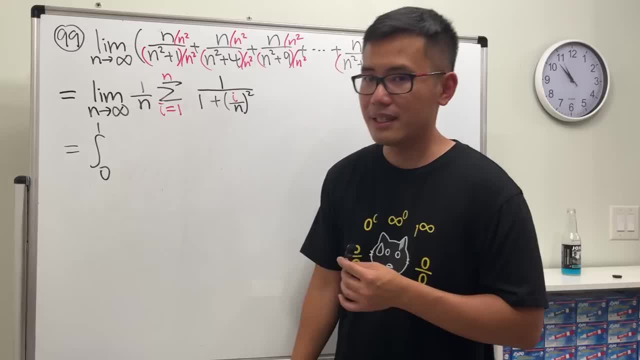 one over n and then one i over n. right, so this is good. this becomes the integral. so this is good. this becomes the integral. so this is good. this becomes the integral of going from zero to one, of going from zero to one, of going from zero to one. the function is one over one plus x. 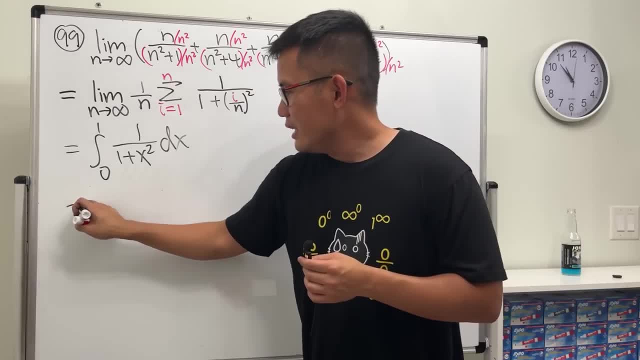 the function is one over one plus x, the function is one over one plus x squared, dx. integrating this, we get inverse tension. integrating this, we get inverse tension. integrating this, we get inverse tension because the derivative inverse tension, because the derivative inverse tension, because the derivative inverse tension is one over one plus x squared. and then 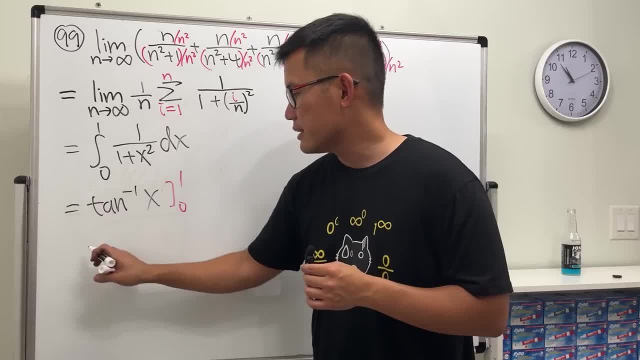 is one over one plus x squared, and then is one over one plus x squared, and then we plug in, plug in, we plug in, plug in, plug in, we plug in, plug in, plug in. one in here: inverse tension of one. one in here: inverse tension of one. 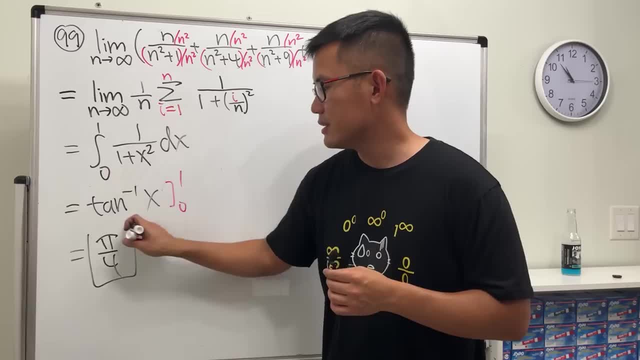 one in here. inverse tension of one is pi over four. plugging zero is pi over four. plugging zero is pi over four. plugging zero is zero. so this right here is, it is zero. so this right here is, it is zero. so this right here is it. that's number 99. 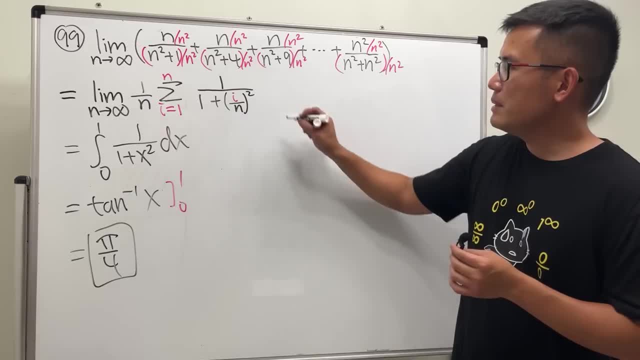 that's number 99. that's number 99, so cool, huh, so cool huh, so cool huh. and you know what? then let me let me, and you know what? then let me let me, and you know what? then let me let me actually write it down right here, this: 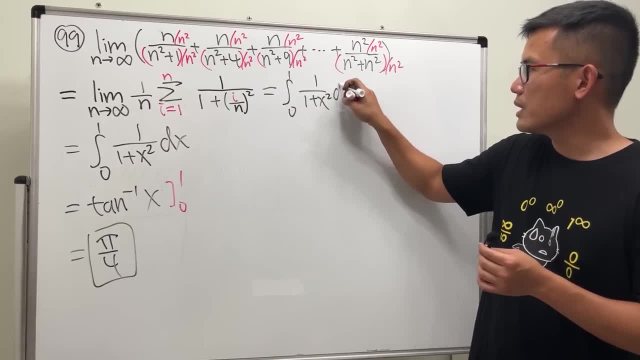 actually write it down right here: this actually write it down right here: this is zero to one, is zero to one, is zero to one. one over one plus x squared. one over one plus x squared. one over one plus x squared. and this is just inverse tangent, and this is just inverse tangent. 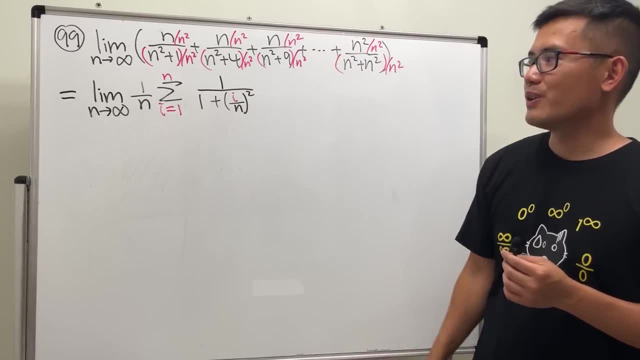 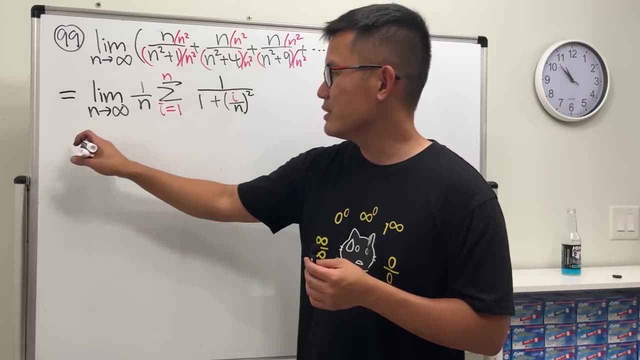 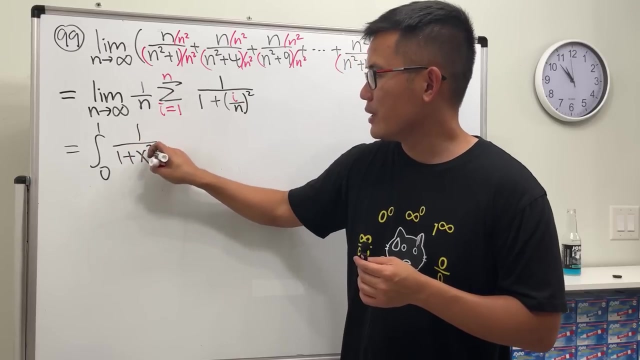 this is 3 square over n square, so on, so on, so on, good, all right. 1 over n, and then 1 i over n, right, so this is good. this becomes the integral of going from 0 to 1. the function is 1 over 1, plus x square dx. 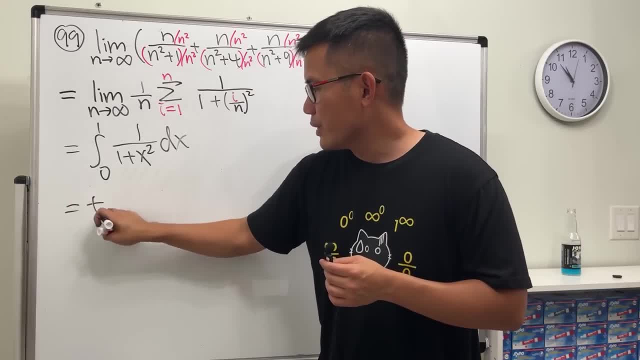 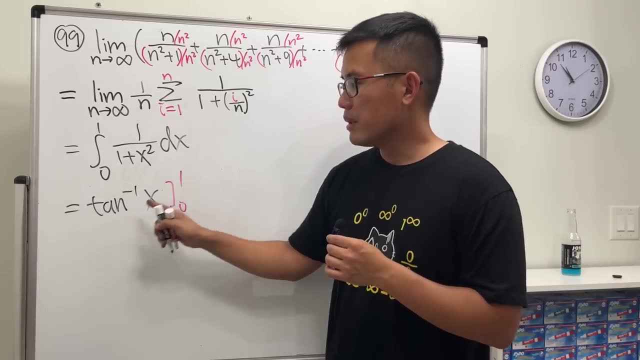 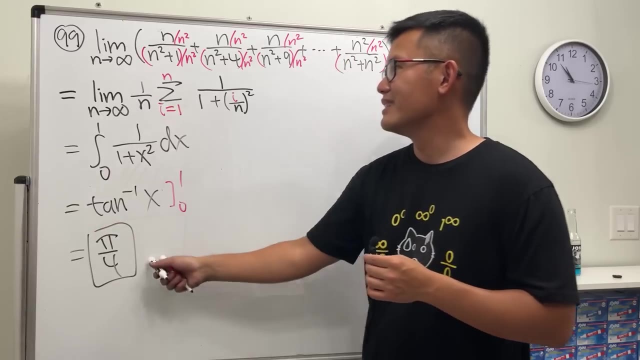 integrating this we get inverse tangent, because the derivative inverse tangent is 1 over 1 plus x square. and then we plug in, plug in, plug in 1 in here, inverse tangent of 1 is pi over 4. plugging 0 is 0. so this right here is it. that's number. 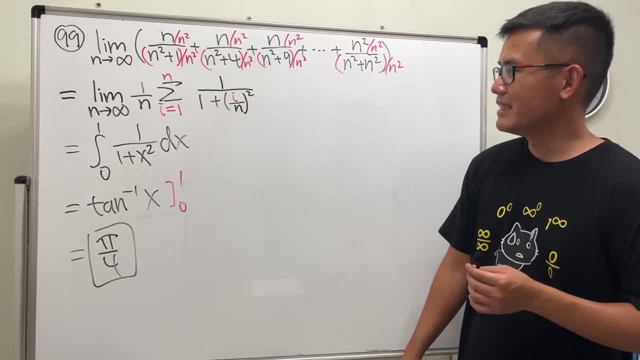 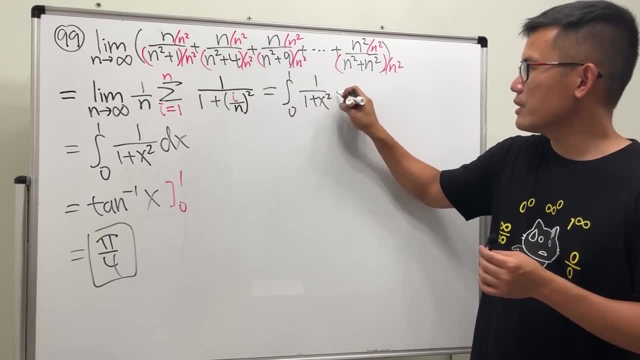 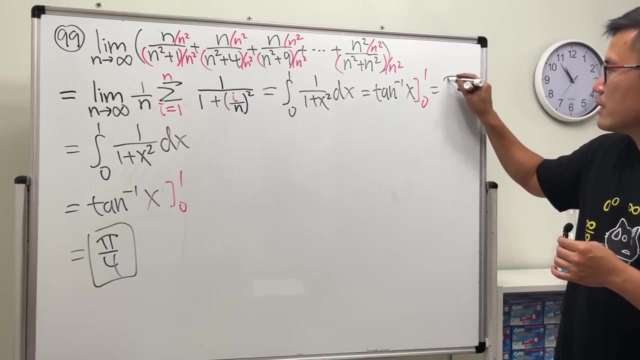 9, 99, so cool, huh, and you know what? then let me let me actually write it down right here. this is 0 to 1, 1 over 1 plus x squared, and this is just inverse tangent of x going from 0 to 1. final answer: pi. 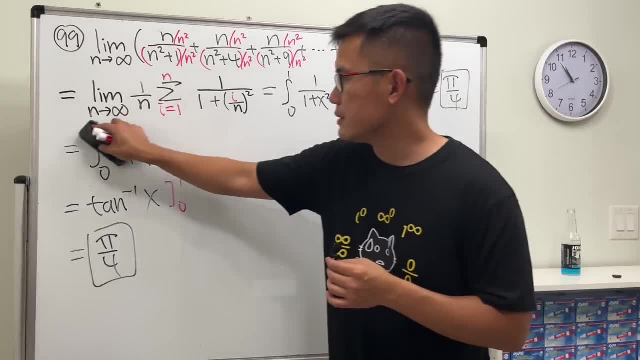 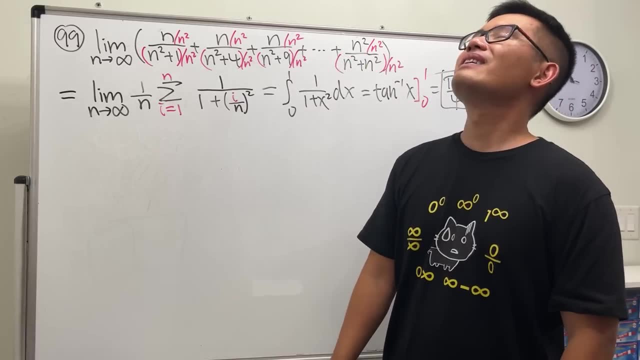 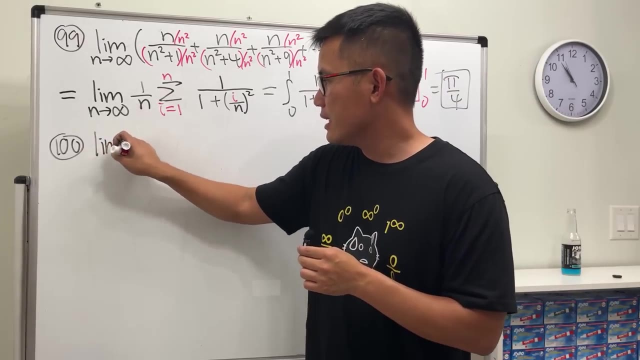 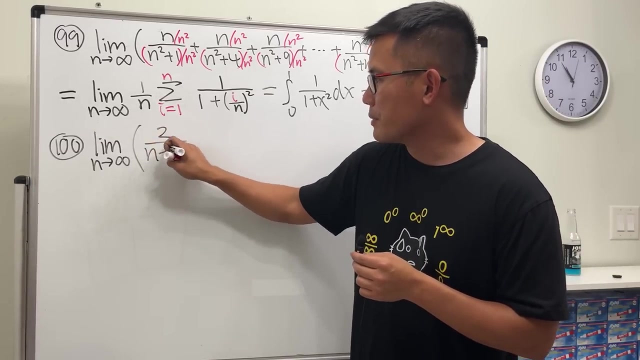 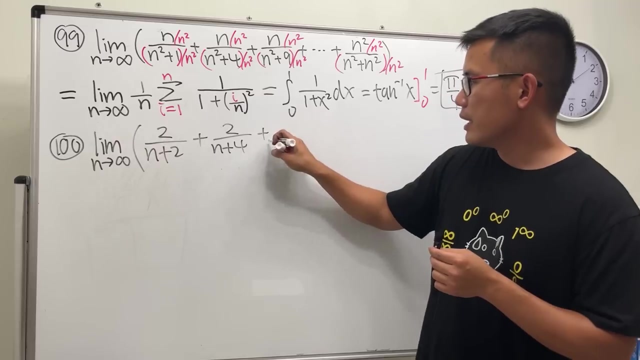 over 4. yeah, because this way i can use the rest right here to do number 100, number 100, all right limit as n goes to infinity. here we have. this marker is the final trial too. it's just two warming side here: 2 over n plus 2, and then 2 over n plus 4, and then 2 over n plus 6. 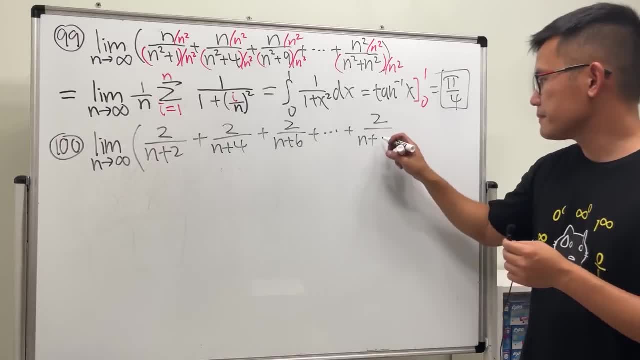 2 over n plus 2n. so quite similar, huh. 2 over n plus 2n, 1 over m plus 1, 1 over n, and so on to infinity. q is equal to 1 over 1 over m plus 2, and then 2 over n plus. oui, oui, ici. voile произ港 là n au astuce de vraiment quite similar, huh呢, if you try to substitute n into n, is everytime the journey goes along two And the order is same. so this is aớaminè model of 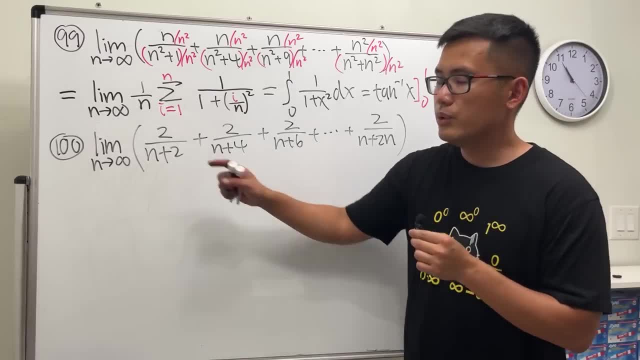 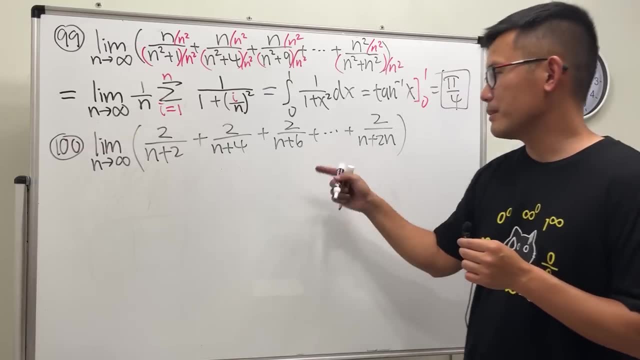 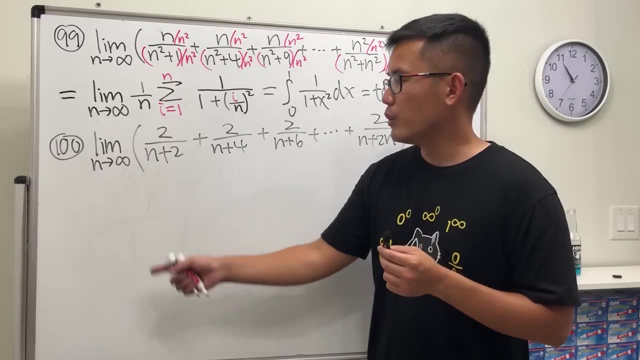 huh, this time we have to recognize that two is the same as two times one, um. and then this right here is the same as two times two, and then two times three, and so on. so maybe we can just divide the top and bottom by n, just like what we did earlier, yes, or you can just factor out the n. 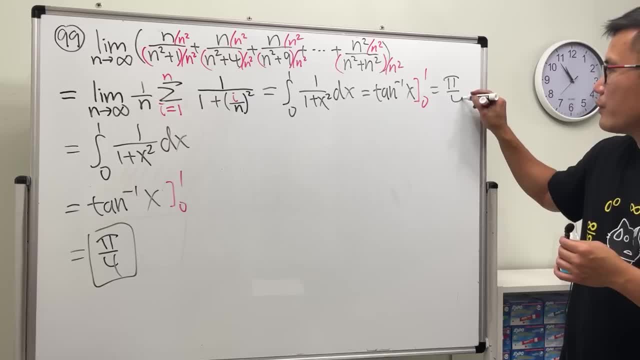 and this is just inverse tangent of x going from zero to one final answer, of x going from zero to one final answer. pi over four. yeah, because this way i can pi over four. yeah, because this way i can pi over four. yeah, because this way i can use the wrist right here to do number. 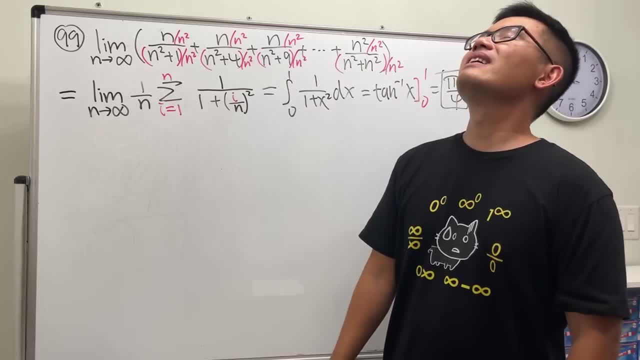 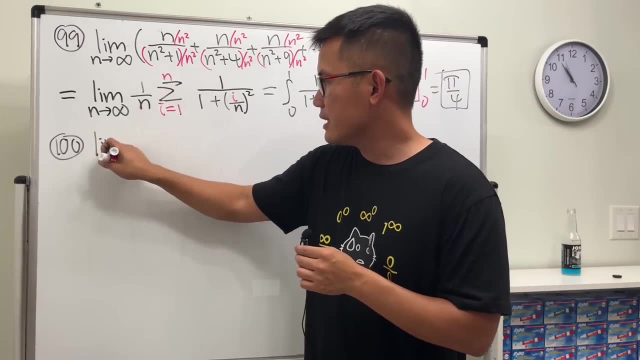 use the wrist right here to do number. use the wrist right here to do number 100. number 100. right limit as n goes to infinity. right limit as n goes to infinity. right limit as n goes to infinity. here we have that this marker is about. here we have that this marker is about. 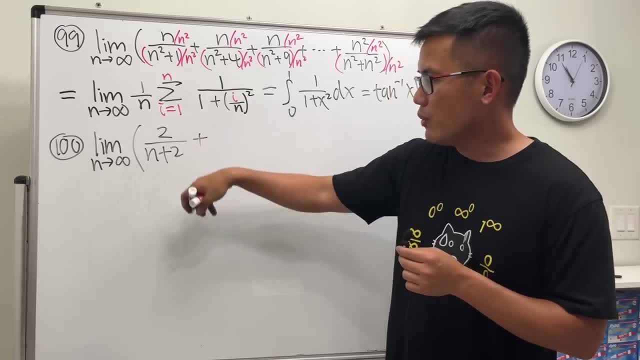 here we have that this marker is about to try out too. to try out too, to try out too. it's just too warm inside here. it's just too warm inside here. it's just too warm inside here. two over n plus two, and then two over n plus two, and then 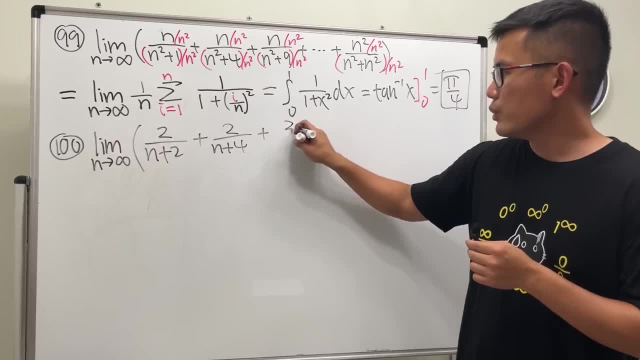 two over n plus two, and then two over two over n plus two, and then two over n plus four, and then two over n plus four, and then two over n plus four, and then two over n plus six, n plus six, n plus six. two over n plus. 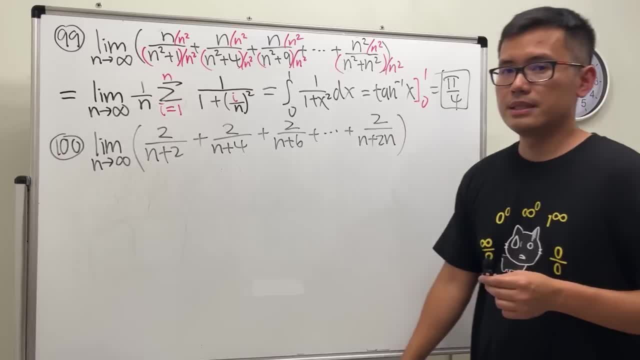 two over n, plus two over n plus two n. so quite similar huh two n. so quite similar huh two n. so quite similar huh. this time we have to recognize that two. this time we have to recognize that two. this time we have to recognize that two is the same as two times one. 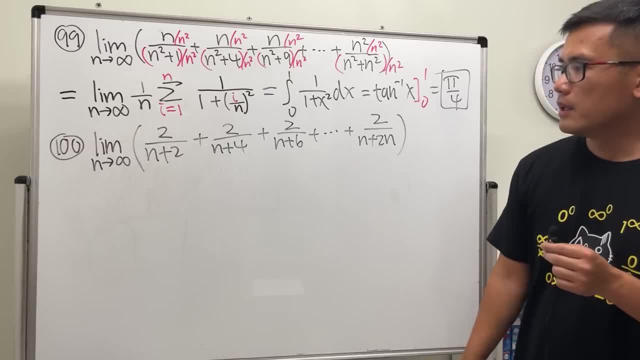 is the same as two times one, is the same as two times one um. and then this right here is the same um. and then this right here is the same um. and then this right here is the same as as as two times two, and then two times three. 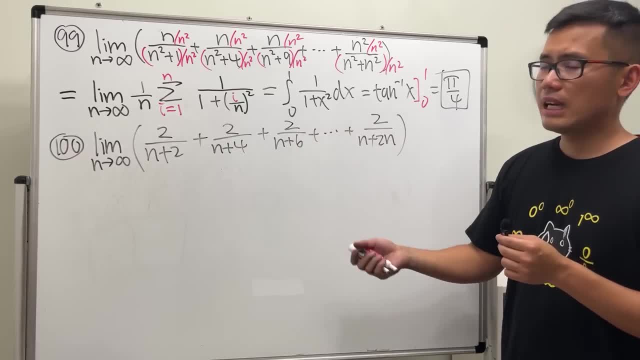 two times two and then two times three, two times two and then two times three, and so on, so and so and so. maybe we can just divide the top, and maybe we can just divide the top, and maybe we can just divide the top and bottom by n, just like what we did earlier. 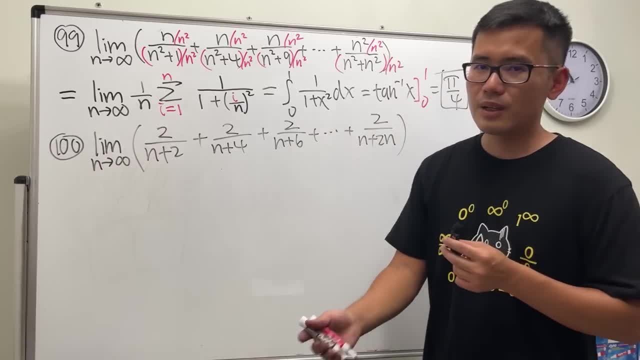 bottom by n, just like what we did earlier. bottom by n, just like what we did earlier. yes, or you can just factor out the end, yes, or you can just factor out the end, yes, or you can just factor out the end from the bottom. so depends on how you. 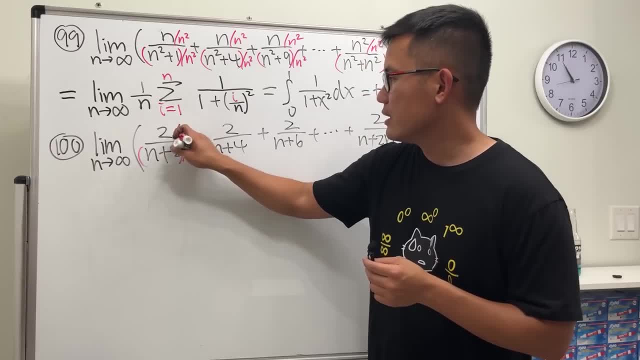 from the bottom. so depends on how you from the bottom. so depends on how you like to look at it. perhaps let's divide like to look at it. perhaps let's divide like to look at it. perhaps let's divide everybody by n, everybody by n, everybody by n. it's more consistent than what we did. 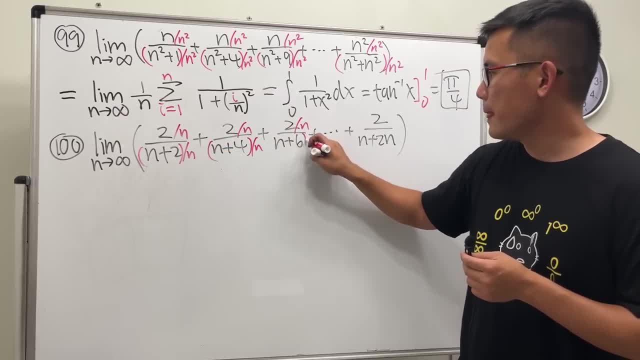 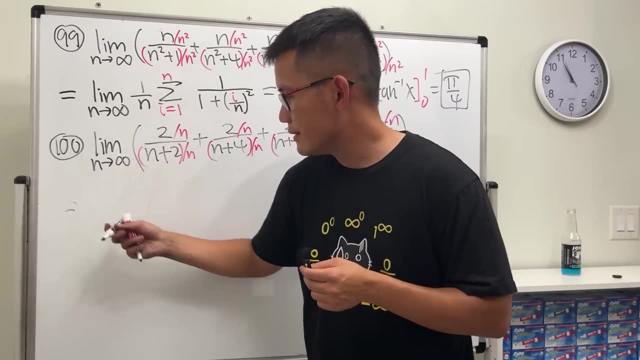 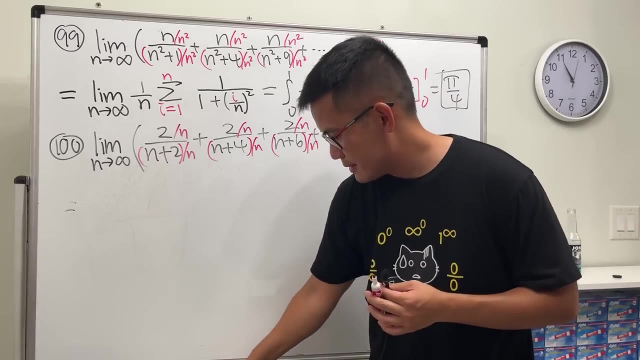 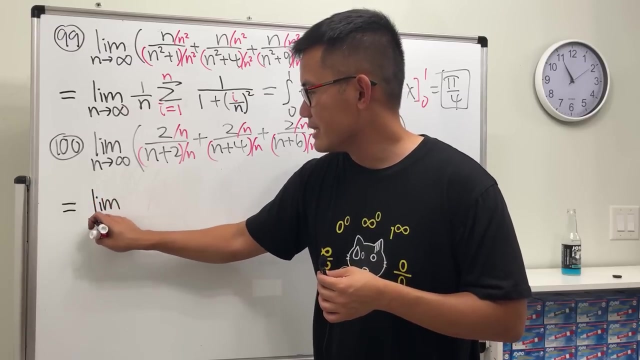 it's more consistent than what we did. it's more consistent than what we did earlier, so earlier, so earlier. so let's do that: perfect, perfect, perfect, so perfect. so this right here is the limit as n goes. so this right here is the limit as n goes. 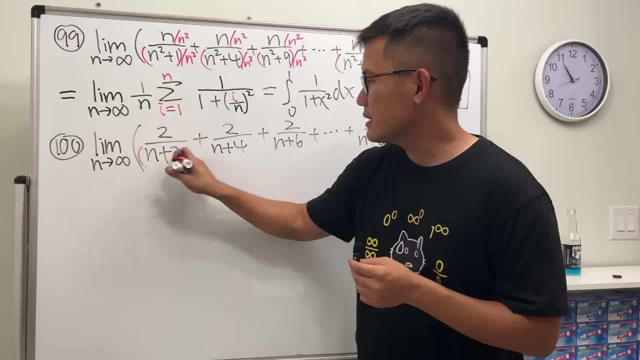 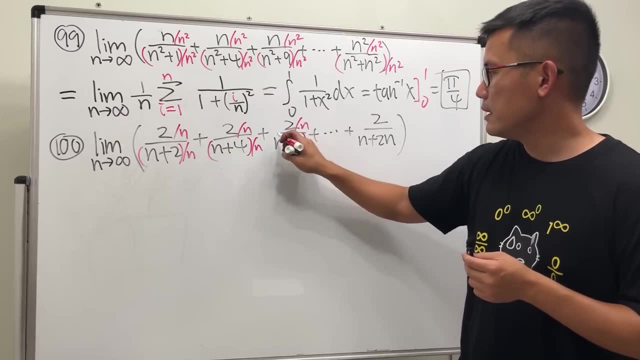 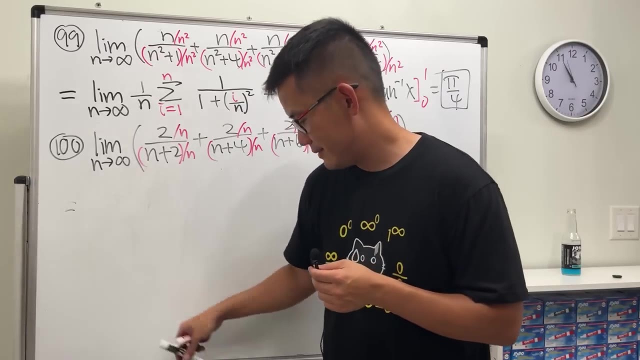 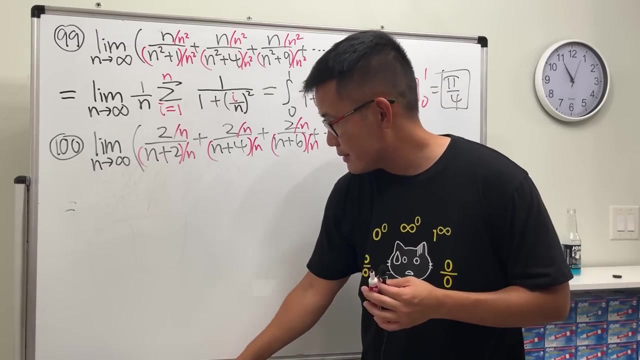 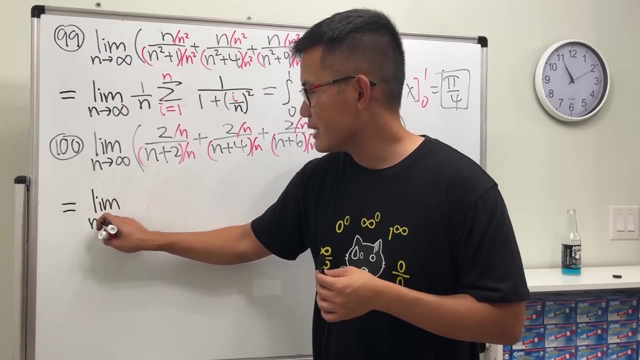 from the bottom. so depends on how you like to look at it. perhaps let's divide everybody by n. it's more consistent than what we did earlier, so let's do that. perfect. so so this right here is the limit, as n goes to infinity. and then we have 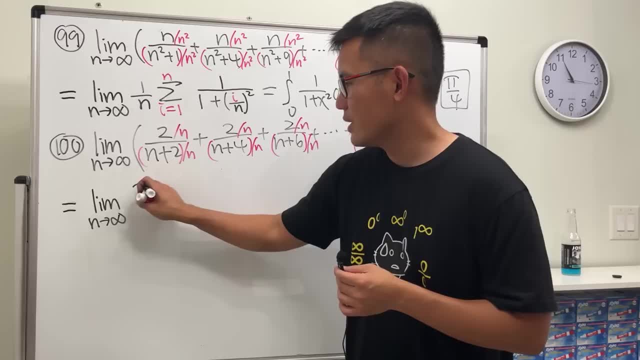 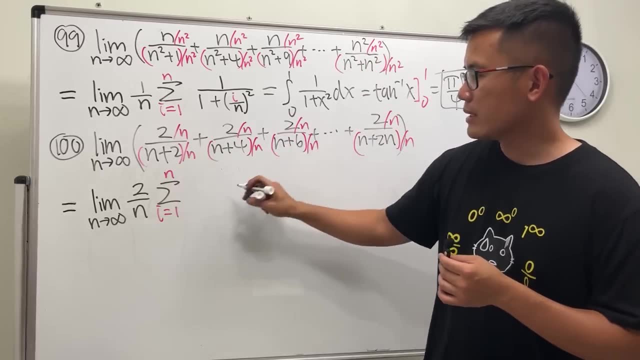 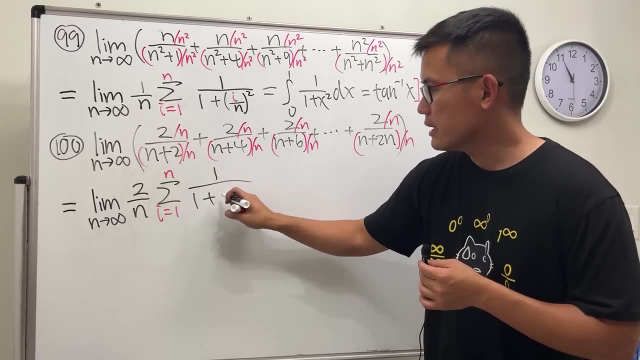 here is the limit, as n goes to infinity. and then we have our 2 over n. let's put that right here. sum i goes from 1 to n, and then now on the top it's just 1, and then we have 1,, right, and then I'm going to write it as plus and we: 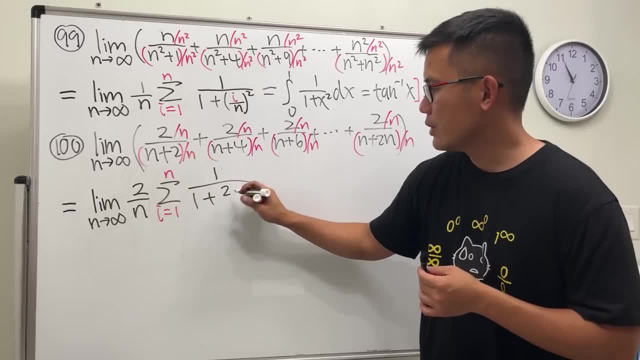 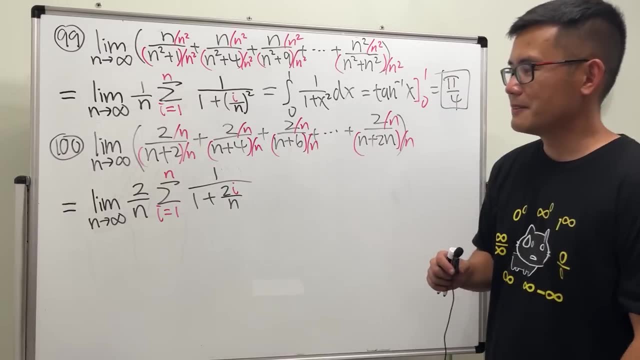 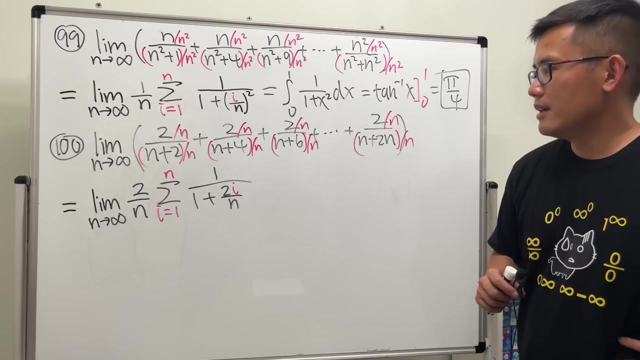 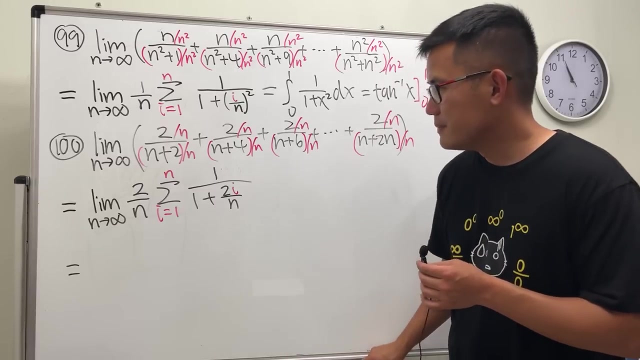 have. this is like 2i. yeah, 2i over n. yes, so it's like this: yeah, is it? yes, yes, yes, yes, okay. so yeah, here we have the integral going from 0 to 2.. 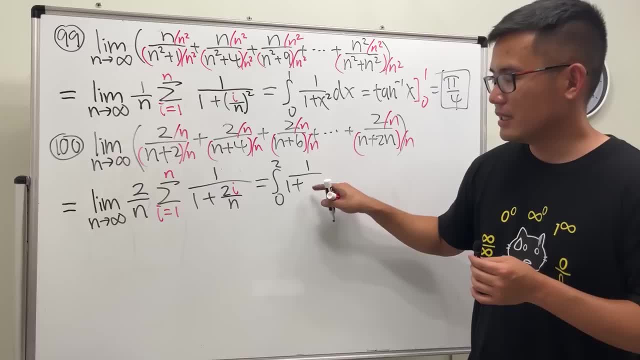 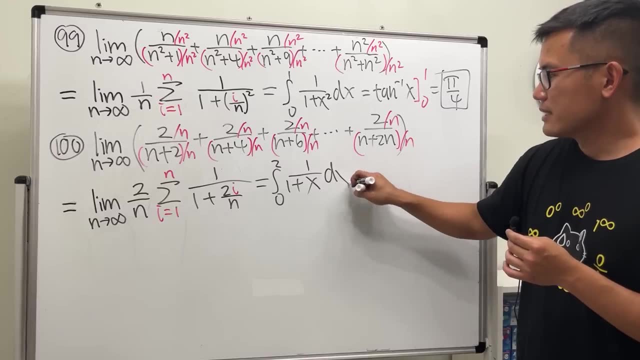 And then the function is 1 over 1 plus is x or 2x. x match right, so x. okay, dx, integrating this is ln of 1 plus x. we don't need the absolute value, because everything. 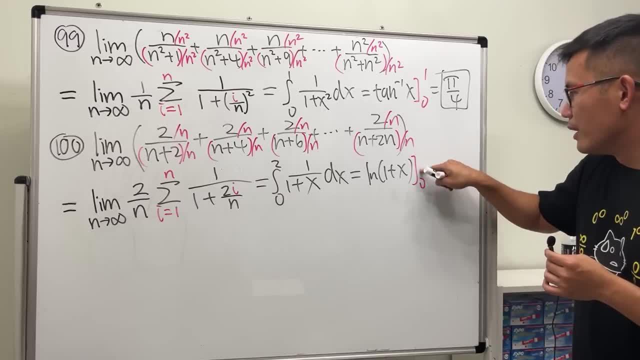 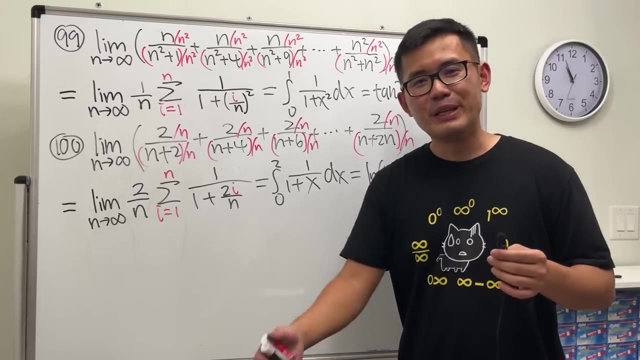 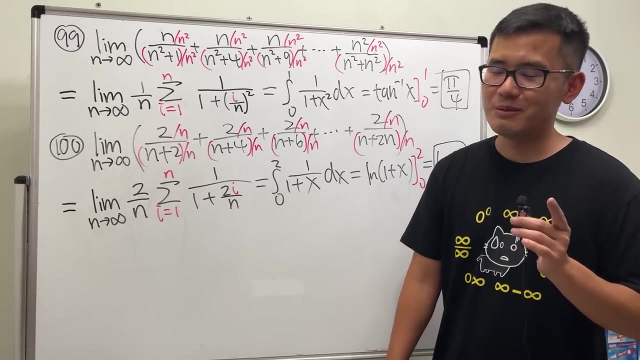 is positive. ladies and gentlemen, plugging 2, we get ln 3,. plugging 0, ln 1 is 0, final answer: ln 3.. 100 limits. there you have it. you know it. I don't just do 100 limits. 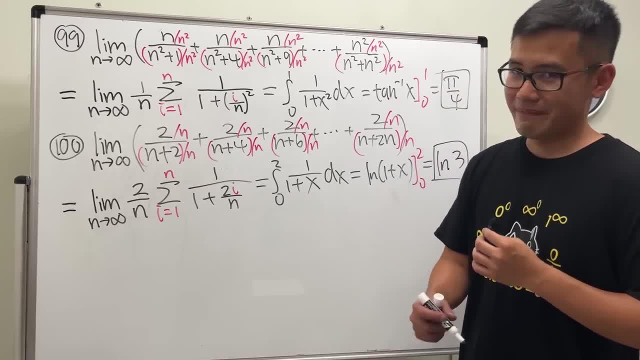 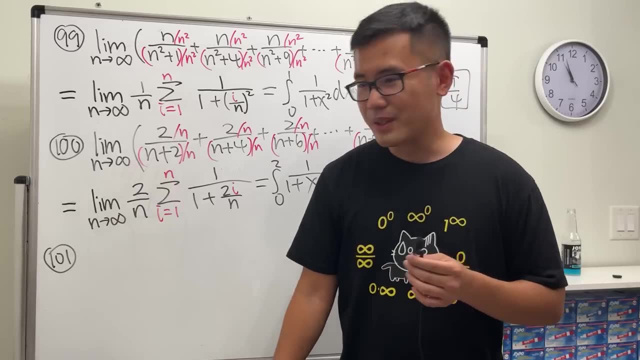 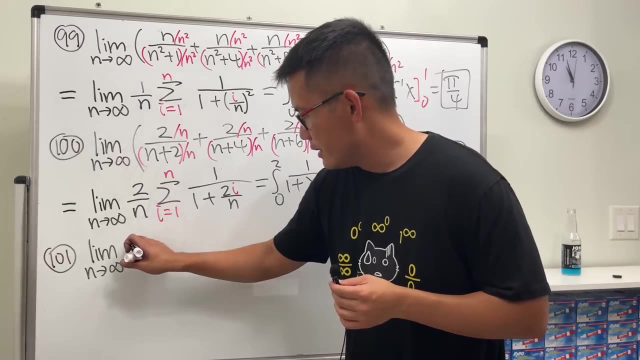 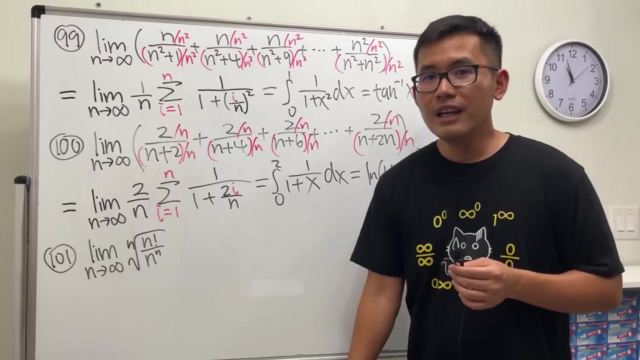 Let's see if we can fit in number 101 here as well. yes, of course. alright, question number 101, what's the question? Limit as n goes to infinity. and then we have, Okay, The nth root of n, factorial over n to the nth power. 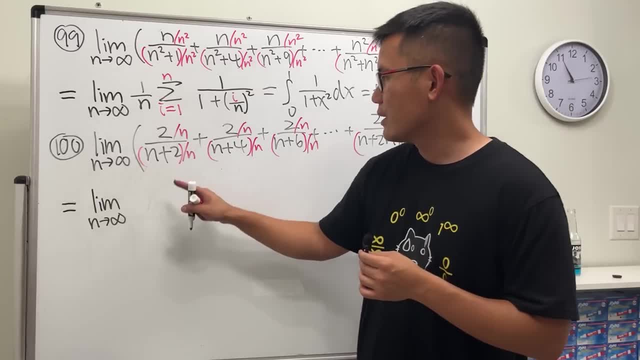 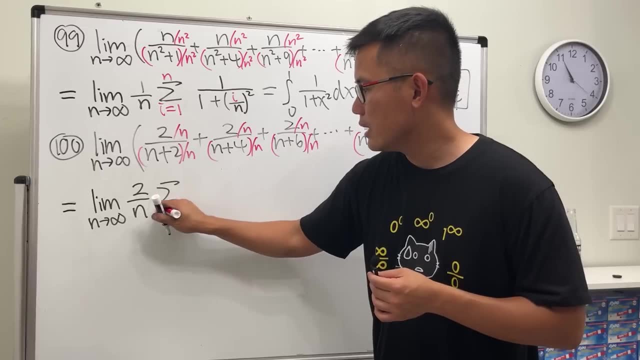 so this, right here, is the limit, as n goes to infinity, to infinity, to infinity, and then we have our, and then we have our, and then we have our 2 over n. let's put that right here: sum, i sum, i sum. i goes from 1 to n, and then now on the. 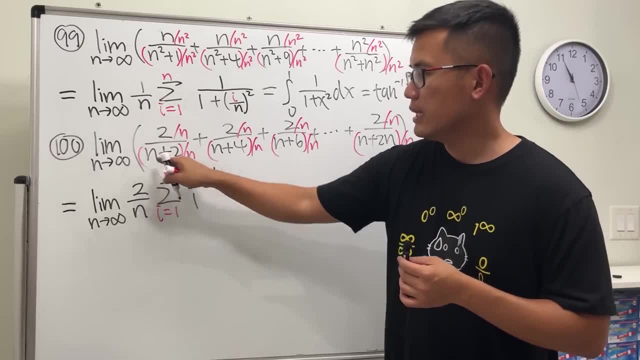 goes from 1 to n, and then now on the goes from 1 to n, and then now on the time: it's just one time, it's just one time, it's just one. and then we have one right, and then, and then we have one right, and then. 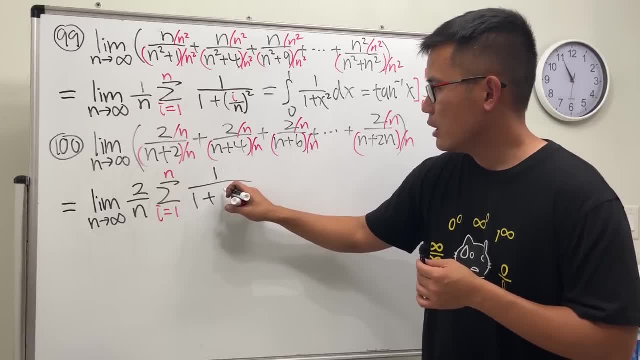 and then we have one right and then i'm going to write it as plus, and we, i'm going to write it as plus, and we, i'm going to write it as plus, and we have, have, have, this is like 2i, yeah, 2i. 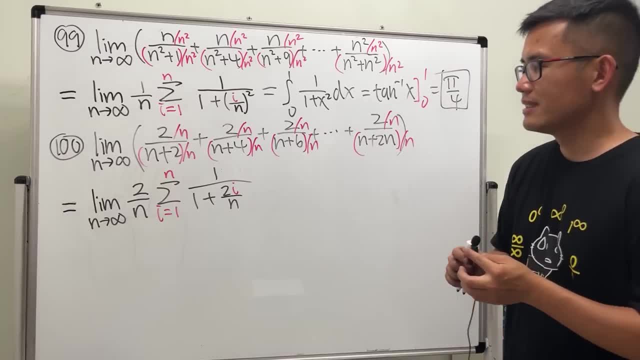 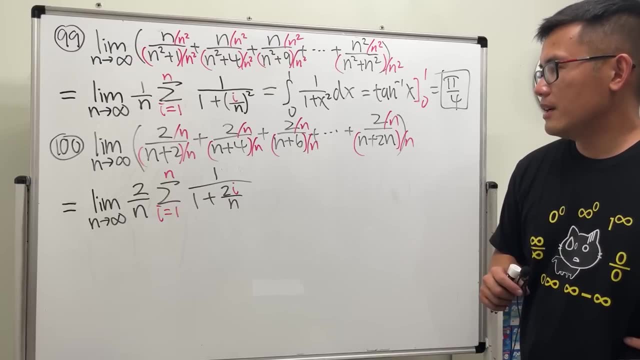 this is like 2i, yeah, 2i. this is like 2i, yeah, 2i, over and over and over, and yes, so it's like this, yes, so it's like this, yes, so it's like this. yeah is it yes, yes, yes, yes, okay, so yeah. 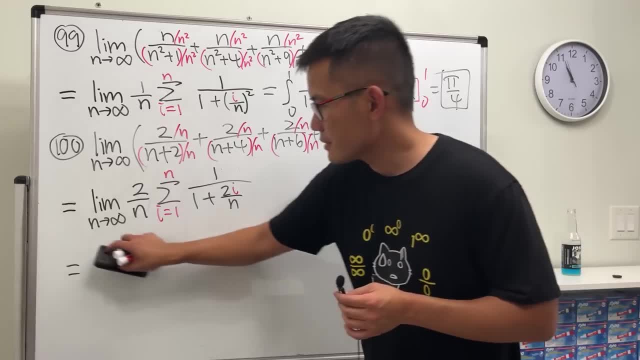 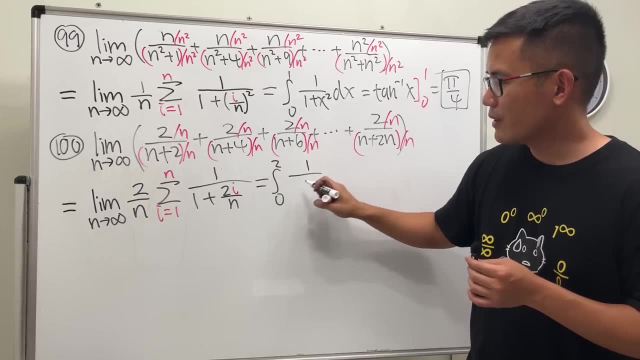 yes, yes, yes, okay, so yeah, yes, yes, yes, okay. so yeah, here we have here. we have here we have the integral going from zero to two. integral going from zero to two. integral going from zero to two, and then the function is one over one plus and then the function is one over one plus. 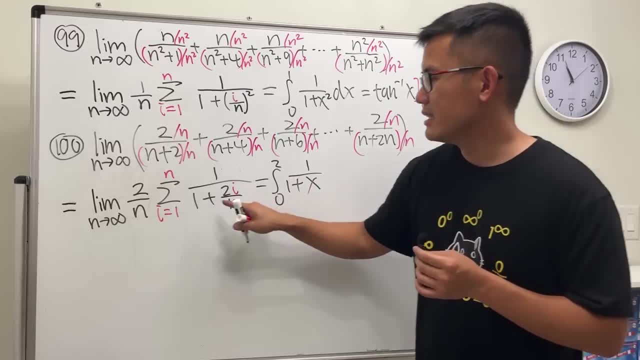 and then the function is one over one plus: is x or 2x, is x or 2x, is x or 2x, x, x, x. match right. so x. match right so x. match right. so x, okay, the x. okay, the x, okay, the x. integrating this is ln of one plus x. we. 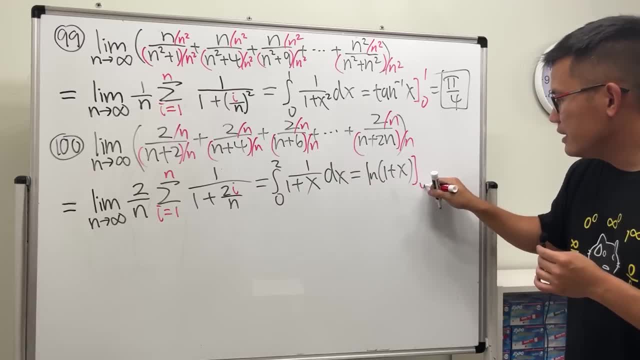 integrating this is ln of one plus x. we integrating this is ln of one plus x. we don't need the absolute value, because don't need the absolute value, because don't need the absolute value, because everything is positive, everything is positive, everything is positive. ladies and gentlemen, 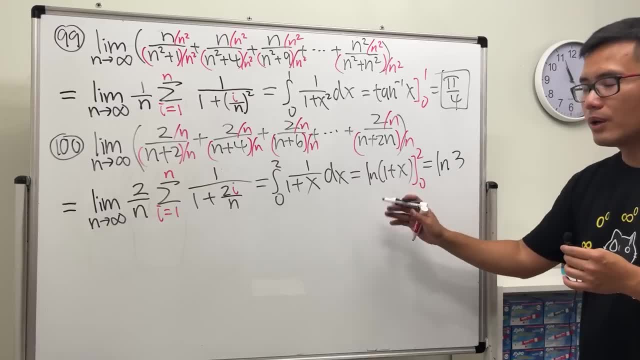 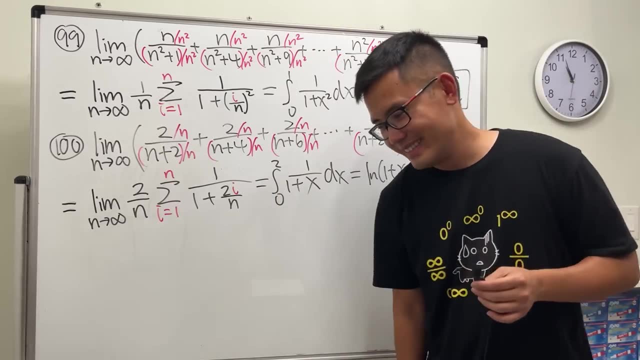 ladies and gentlemen. ladies and gentlemen, plug-in 2: we get ln 3. plug-in 2: we get ln 3. plug-in 2: we get ln 3. plug-in 0: ln 1 is plug-in 0. ln 1 is plug-in 0. ln 1 is 0. final answer: lx3. 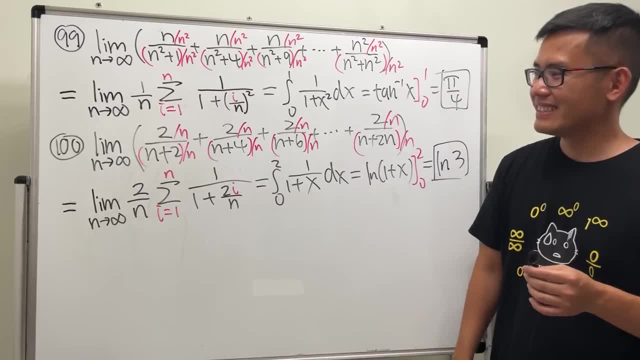 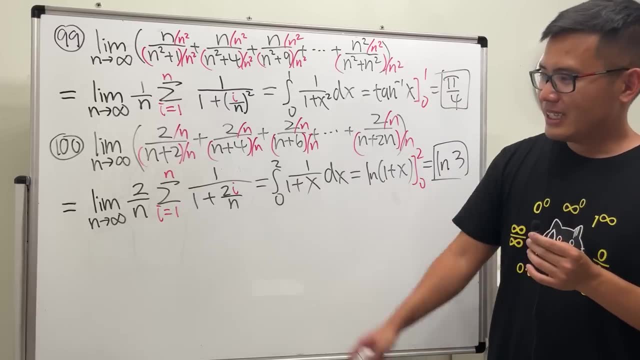 100 limits. there you have it. you know it. i don't just do 100 limits, you know it. i don't just do 100 limits, you know it. i don't just do 100 limits. let's see if we can fill in number 101. 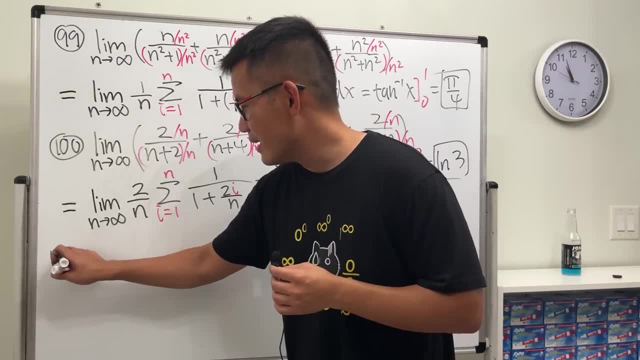 let's see if we can fill in number 101. let's see if we can fill in number 101 here as well. here as well, here as well. yes, of course, all right. yes, of course all right. yes, of course, all right. question number 101. question number 101. 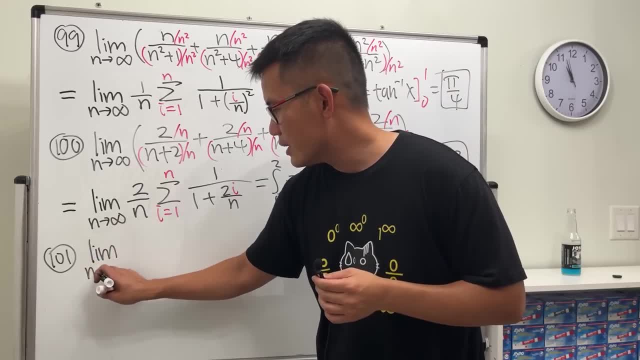 question number 101. what's the question? what's the question? what's the question? limit limit, limit limit as n goes to infinity, and then we have as n goes to infinity, and then we have as n goes to infinity, and then we have the nth root of. 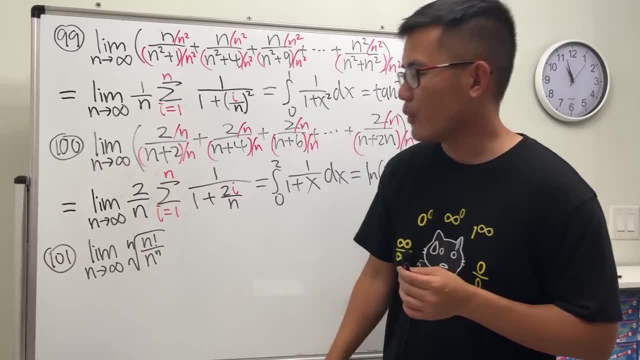 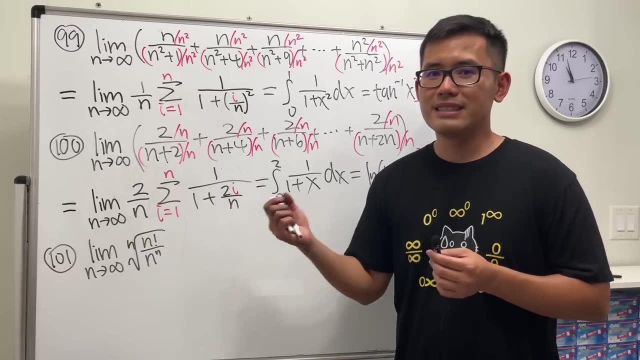 the nth root of the nth root of n factorial over n to the nth power, n factorial over n to the nth power, n factorial over n to the nth power. why is this one number 101? yeah, because why is this one number 101? yeah, because why is this one number 101? yeah, because this right here has the most amount of. 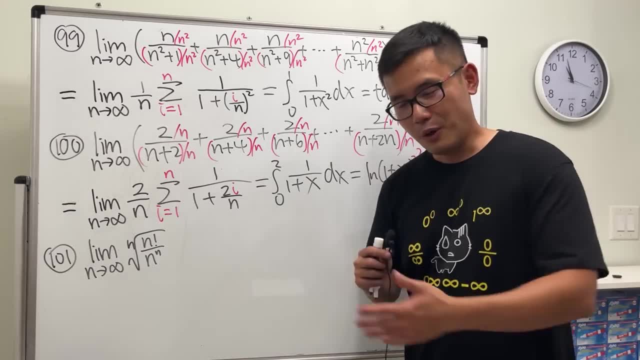 this right here has the most amount of this right here has the most amount of view, view, view, right. i have a video just on this, right. i have a video just on this right. i have a video just on this: over 1 million views, right, my brilliant. 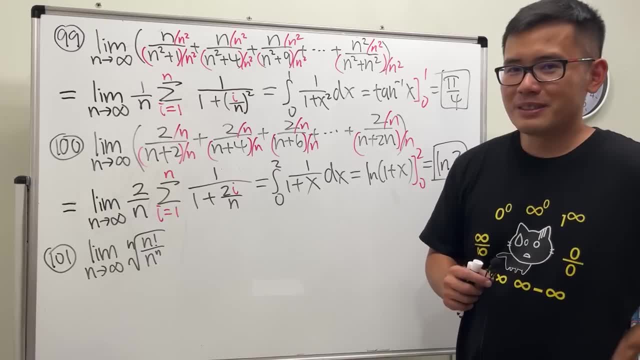 over 1 million views. right, my brilliant over 1 million views. right, my brilliant limit limit limit. yeah, yeah, yeah. thanks to brilliant for sponsoring. thanks to brilliant for sponsoring. thanks to brilliant for sponsoring me for throughout this year. i really me for throughout this year. i really 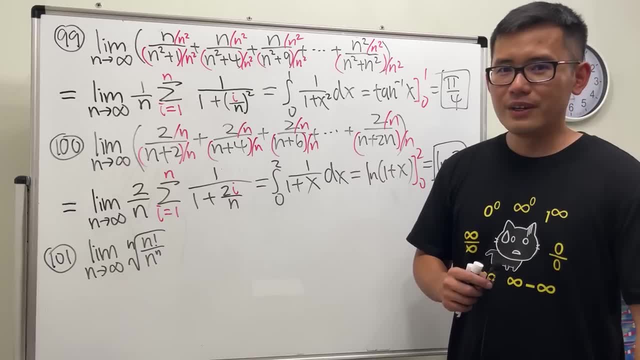 me for throughout this year. i really appreciate everybody's help, appreciate everybody's help, appreciate everybody's help and everybody's watching video, and then all and everybody's watching video, and then all and everybody's watching video, and then all the sponsors that i have. i'm very 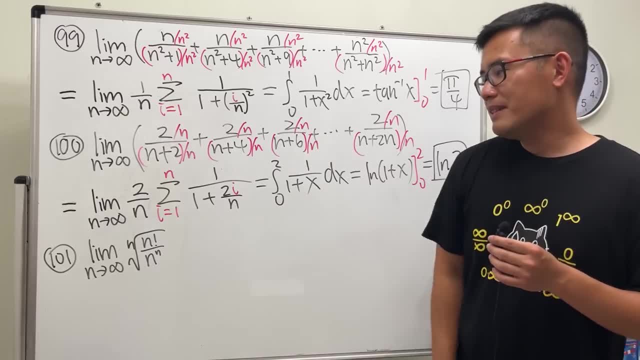 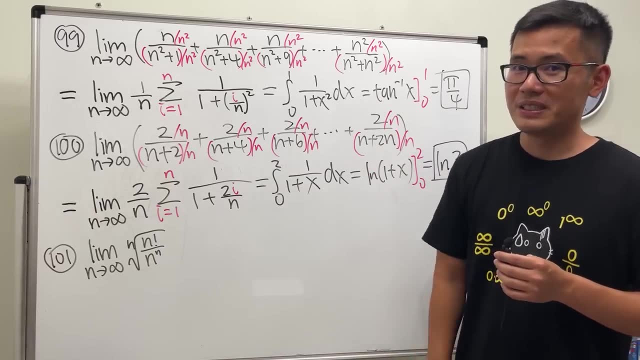 the sponsors that i have. i'm very the sponsors that i have. i'm very grateful. i'm debating to see. i'm debating to see. i'm debating to see if i can, if i can, if i can show you guys two solutions here. do you guys want two solutions? 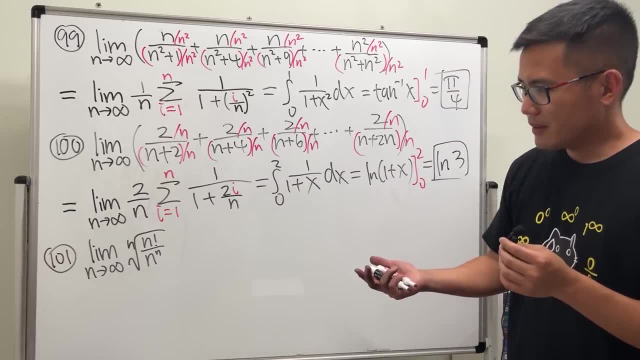 do you guys want two solutions? do you guys want two solutions? i think, just to honor the. i think just to honor the. i think just to honor the, the brilliant limit, the brilliant limit, the brilliant limit. i am going to, i am going to, i am going to do the same thing. 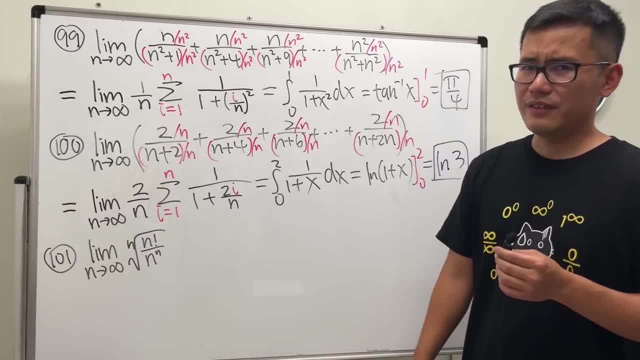 do the same thing. do the same thing, kind of consistent of what we did. let me kind of consistent of what we did. let me kind of consistent of what we did. let me see if i can fit in everything, see if i can fit in everything, see if i can fit in everything. firstly, 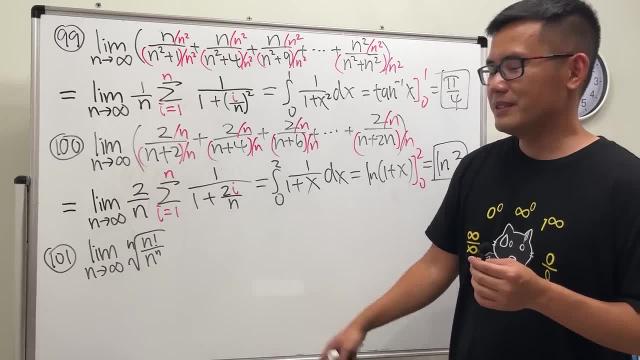 actually, no, i cannot fit in everything. actually no, i cannot fit in everything. actually no, i cannot fit in everything. so, if you want to see the original way, so, if you want to see the original way, so, if you want to see the original way that i stopped this, go ahead and check. 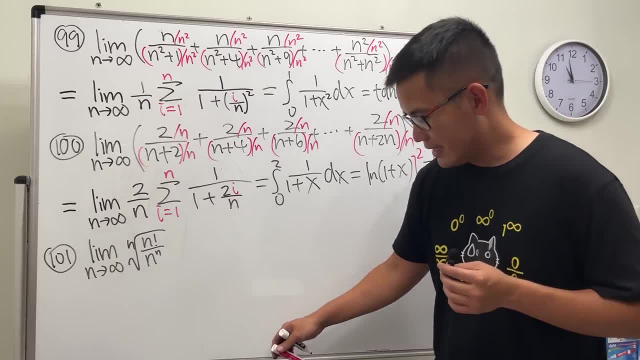 that i stopped this. go ahead and check that i stopped this. go ahead and check out my other video right here. i would out my other video right here. i would out my other video right here. i would like to show you guys, like to show you guys, like to show you guys, another way to solve it. 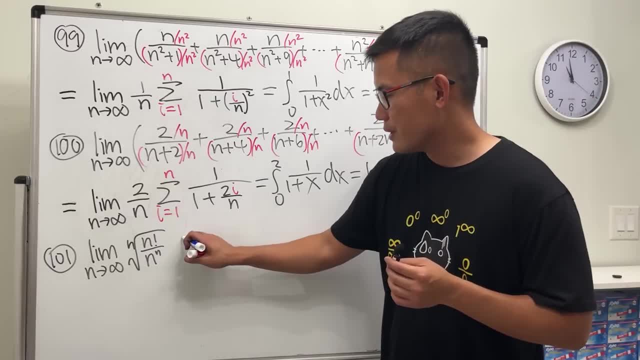 another way to solve it. another way to solve it. this is true. i don't have a place to this is true. i don't have a place to this is true. i don't have a place to prove, so i'll just tell you note. prove, so i'll just tell you note. 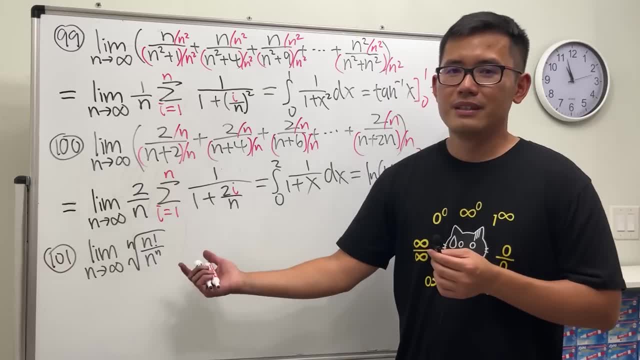 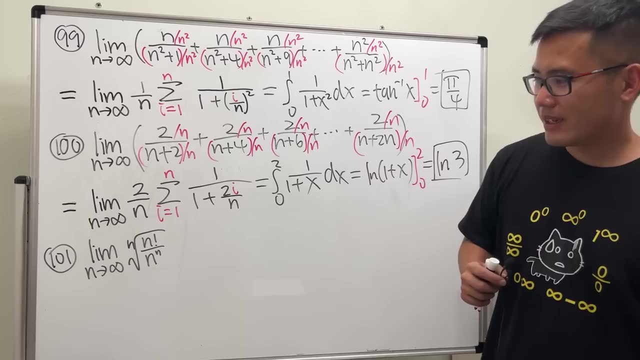 Why is this one number 101?? Yeah, because this right here has the most amount of view, right? I have a video just on this: over 1 million views, right, my brilliant limit. yeah, yeah, thanks to Brilliant for. 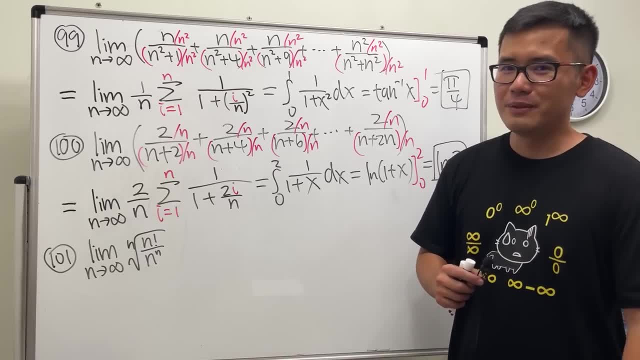 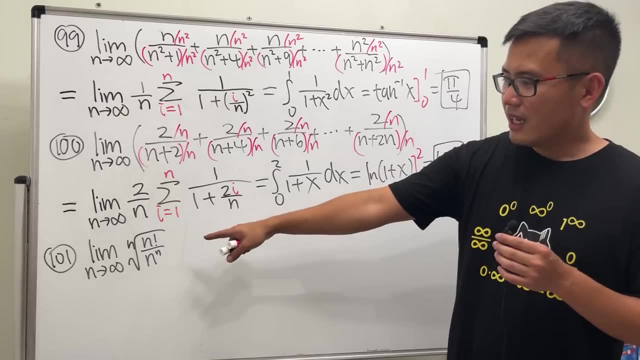 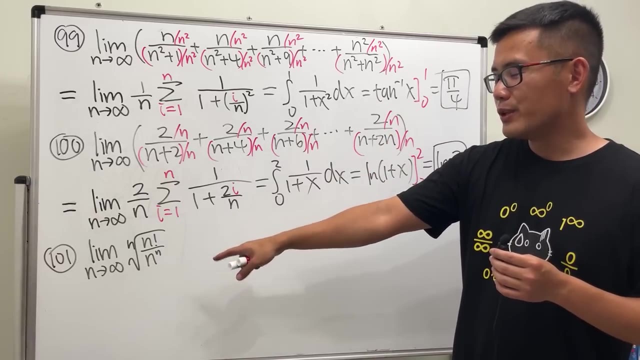 sponsoring me throughout this year. I really appreciate everybody's help and everybody's watching video And all the sponsors that I have. I'm very grateful. I am debating to see if I can show you guys two solutions here. do you guys want two solutions? 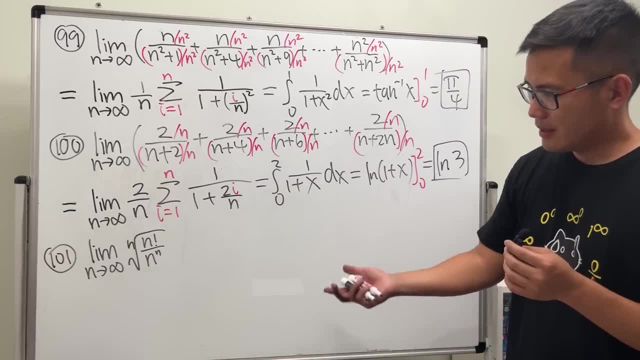 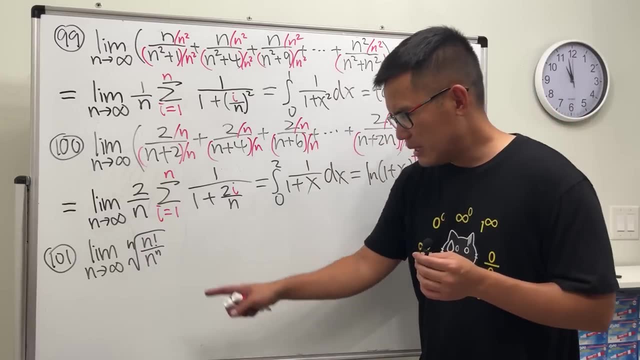 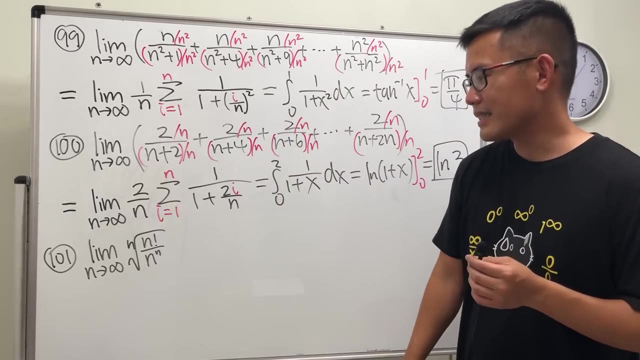 I think just to honor the Brilliant limit, I am going to do the same thing, kind of consistent of what we did. Let me see if I can fit in everything. Okay, Firstly, actually no, I cannot fit in everything. So if you want to see the original way that I solved this, go ahead and check out my other. 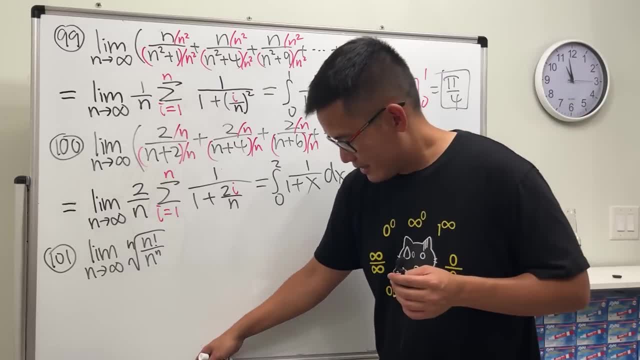 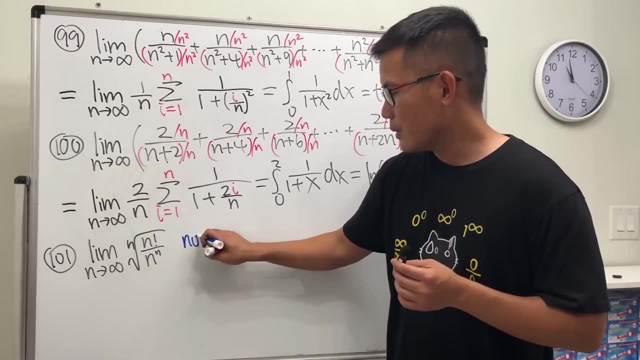 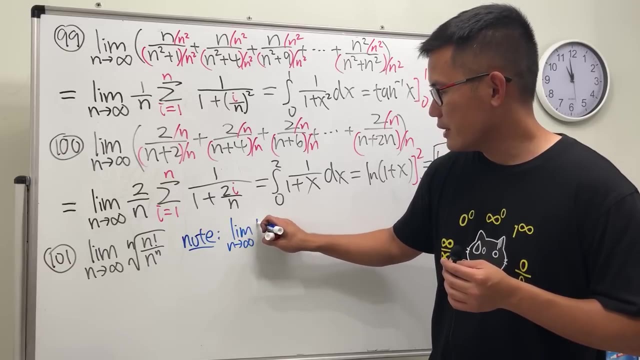 video right here. I would like to show you guys another way to solve it. This is true. I don't have a place to prove, So I'll just tell you. note if we have the limit as n goes to infinity of an nth root. 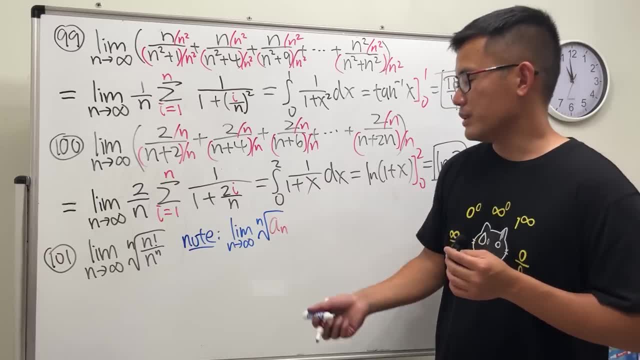 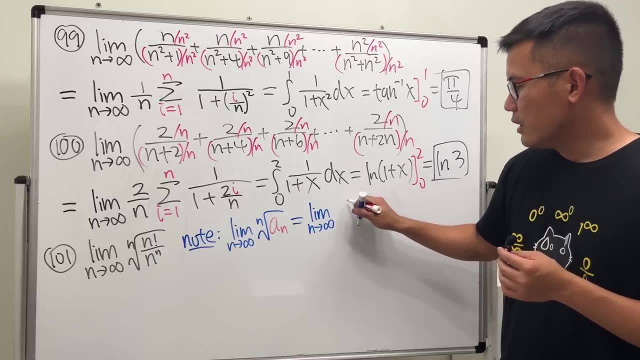 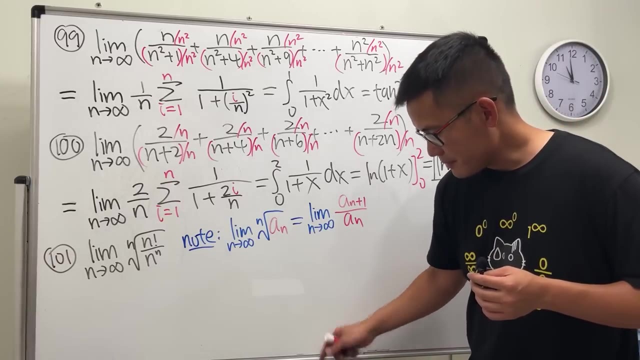 of some sequence. an like this, this right here, it's actually the same as the limit, as n goes to infinity of an plus one over an. yeah, where did I saw this? where did I see this? I saw this on Wikipedia. 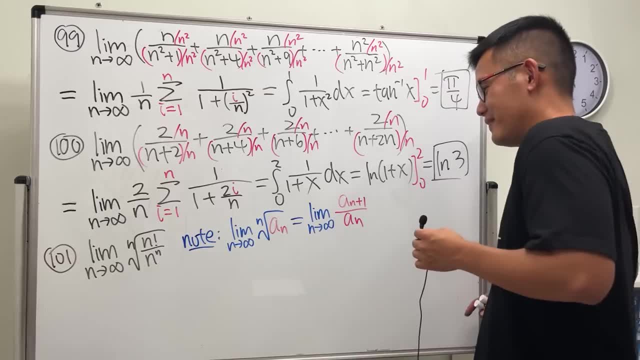 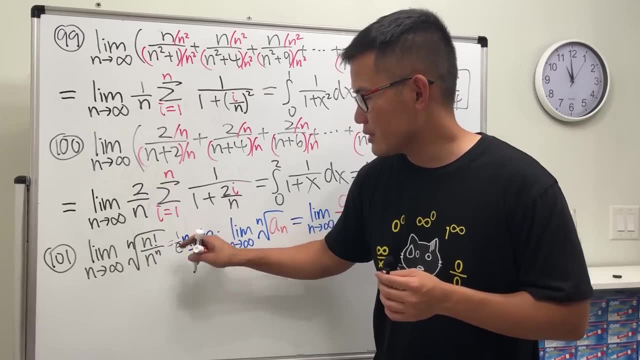 So yeah, this fits this condition. and then I can finish this nicely. Remember the answer that we got from the Brilliant limit is one over e, So keep that in mind. I will show you that this is actually one over e as well. 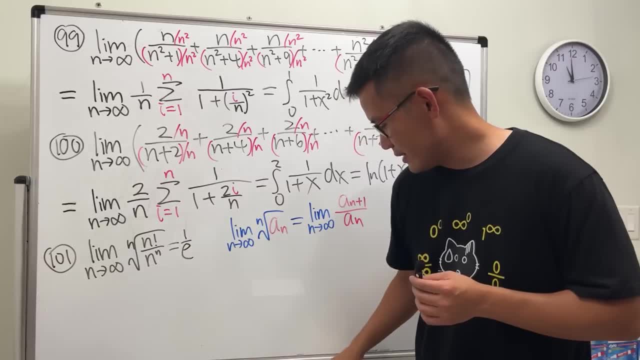 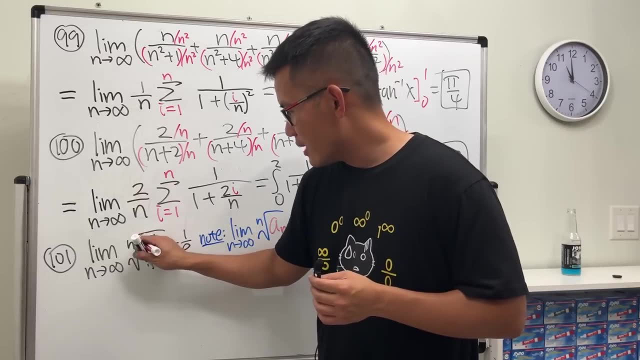 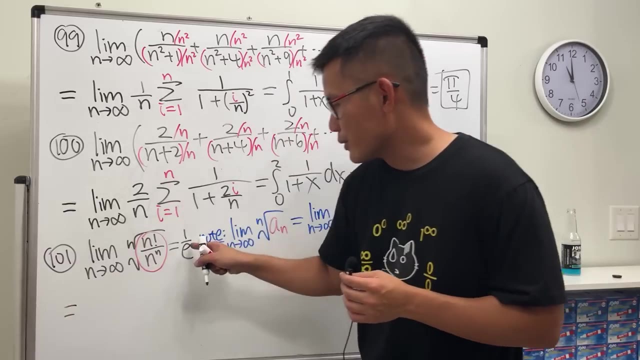 Okay, This is one over e All right, So cool. Now, this right here is our inner limit, so it's just an yeah, So let's just go ahead and check. I don't know this yet. Okay, of course. 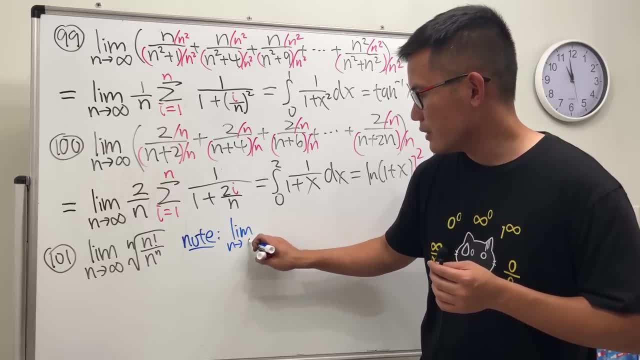 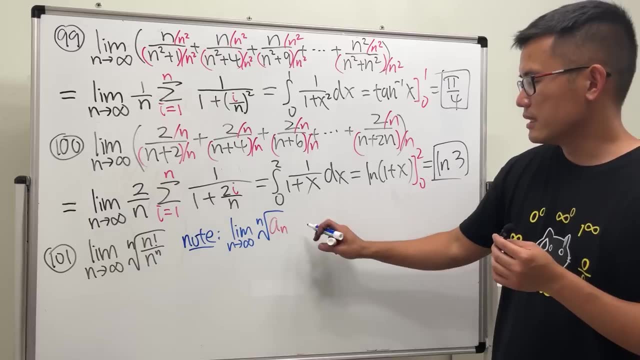 prove. so i'll just tell you note: if we have the limit as n goes to, if we have the limit as n goes to, if we have the limit as n goes to infinity of an nth root of some sequence like a n like this, this right. sequence like a n like this, this right. 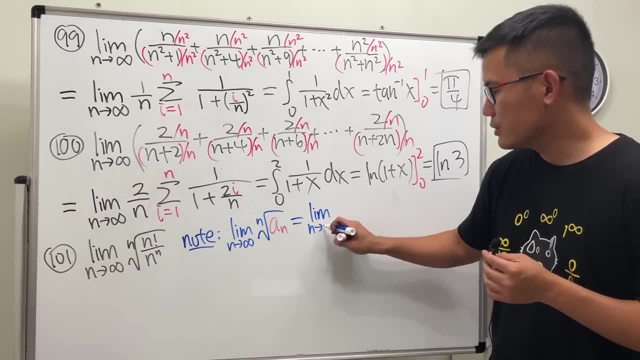 sequence, like a n, like this, this right here. it's actually here. it's actually here, it's actually the same as the limit, as n goes to the same as the limit as n goes to the same as the limit as n goes to infinity, infinity. infinity of a n plus one over a n. 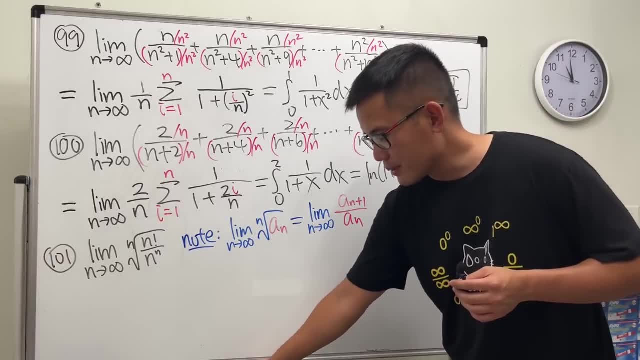 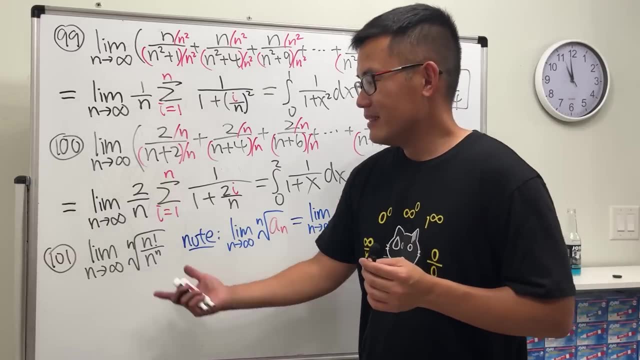 of a n plus one over a n, of a n plus one over a n. yeah, where did i saw this? where did i see? where did i saw this? where did i see? where did i saw this? where did i see this? i saw this on wikipedia. so, yeah, this fits this condition. and then i 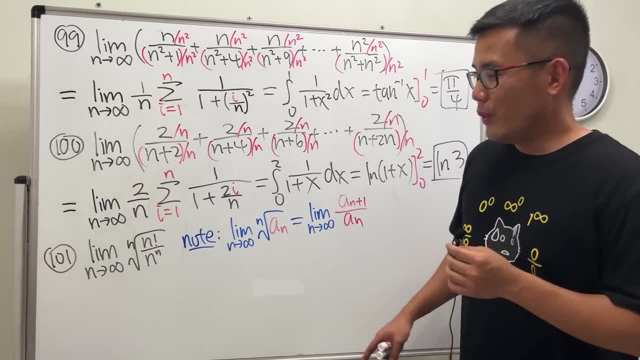 so, yeah, this fits this condition. and then i so yeah, this fits this condition, and then i can finish this, can finish this, can finish this nicely. remember the answer that we got nicely. remember the answer that we got nicely. remember the answer that we got from: the brilliant limit is one over e. 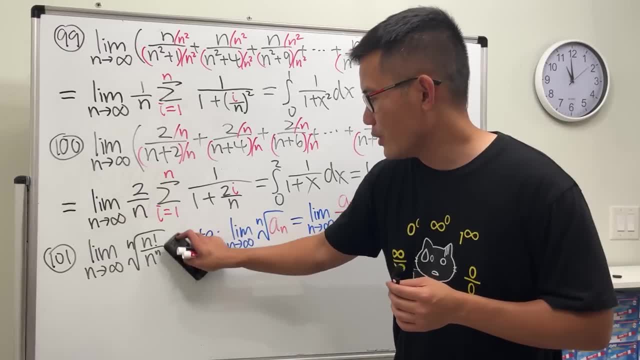 from the brilliant limit is one over e. from the brilliant limit is one over e. so keep that in mind. i'll show you that. so keep that in mind. i'll show you that. so keep that in mind. i'll show you that this is actually one over e as well. 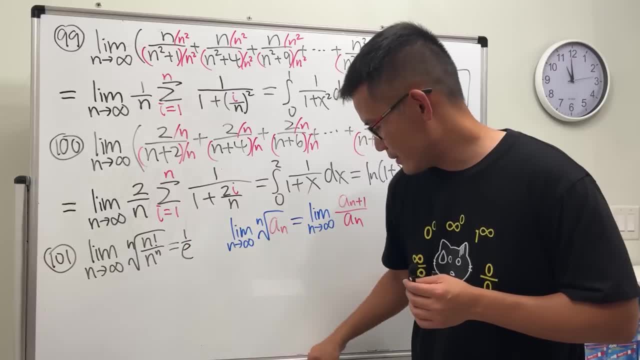 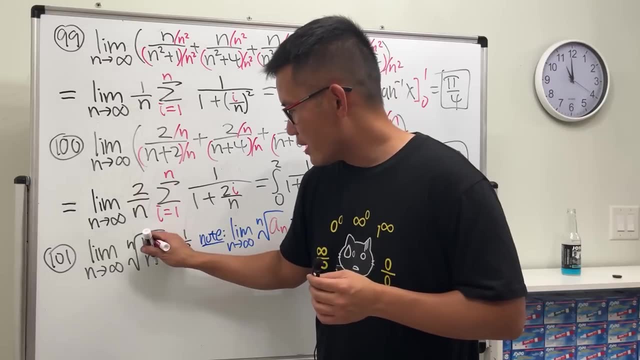 this is actually one over e as well. this is actually one over e as well. okay, this is one over e. okay, this is one over e. all right, so cool now, this right here. cool now, this right here. cool now, this right here. it's our, it's our. 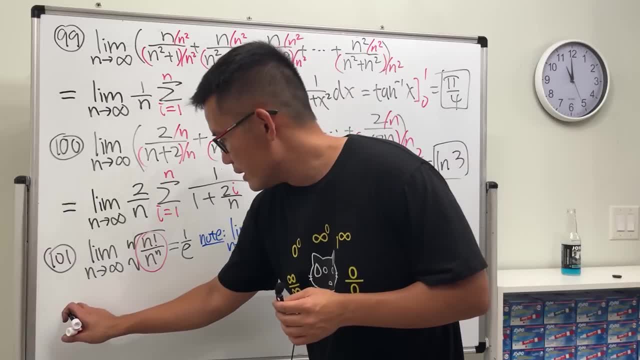 it's our inner limit. so it's just a n. yeah. so inner limit, so it's just a n- yeah. so inner limit, so it's just a n yeah. so let's just go ahead and check, i don't. let's just go ahead and check, i don't. 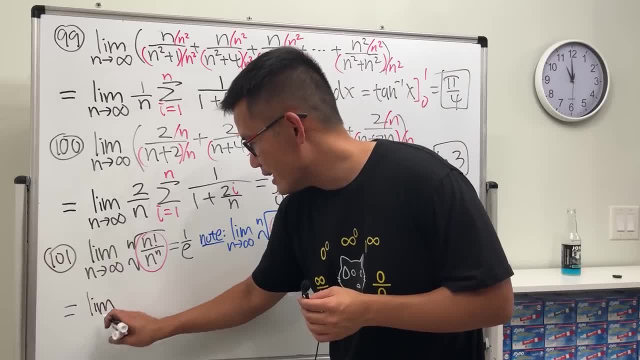 let's just go ahead and check. i don't know this yet okay, of course. so this. know this yet okay, of course. so this. know this yet okay, of course. so this. right here is the limit, right here is the limit, right here is the limit as n goes to infinity. it's like whenever. 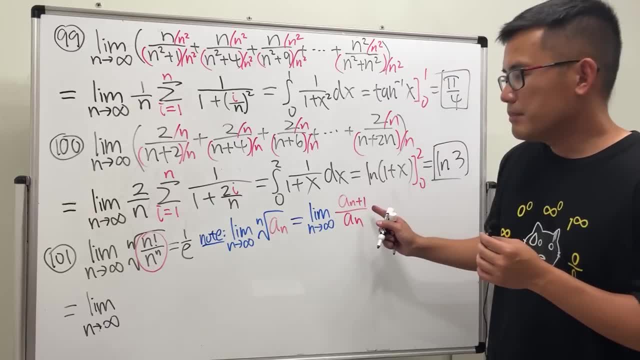 as n goes to infinity. it's like whenever as n goes to infinity. it's like whenever we have the answer, we just look at, we have the answer. we just look at, we have the answer. we just look at the inside and just do a n plus one. 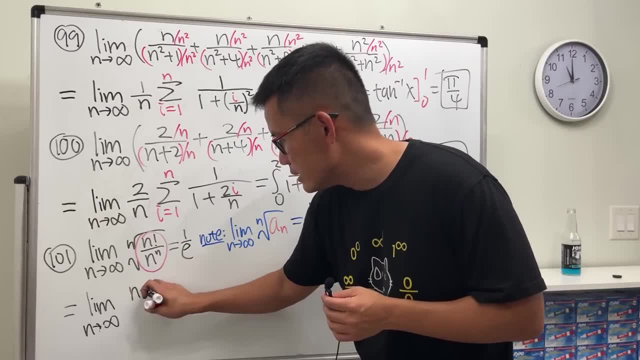 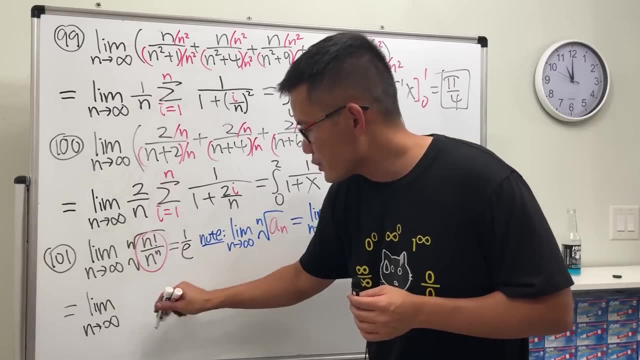 the inside and just do a n plus one the inside, and just do a n plus one, meaning that we do, meaning that we do, meaning that we do n plus one, n plus one, n plus one, and then we factorial that sorry, sorry, sorry, n plus one. so 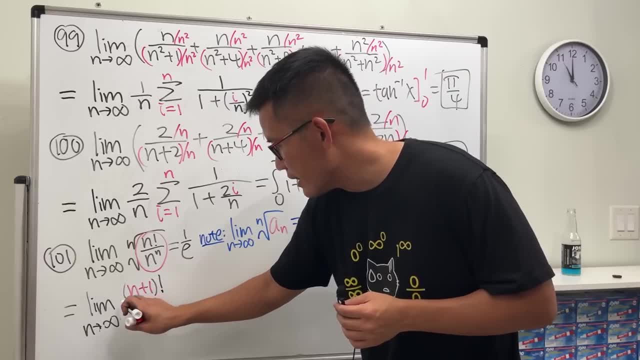 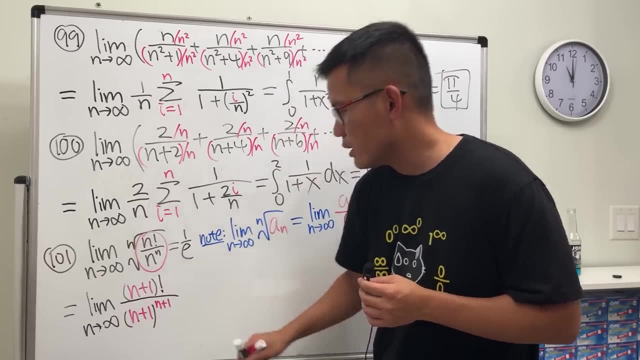 n plus one, so n plus one, so n plus one, n plus one, n plus one factorial that, factorial, that, factorial that, and then, and then, and then, n plus one, n plus one, n plus one. raise to the n plus one power, raise to the n plus one power. 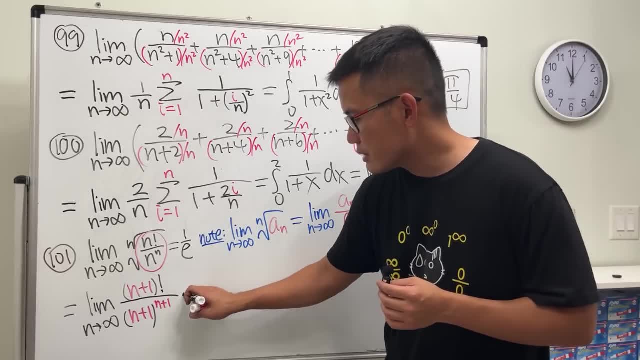 raise to the n plus one power, and then we want to divide it by a n, and then we want to divide it by a n, and then we want to divide it by a n, which is the same as just, which is the same as just, which is the same as just multiply by it's reciprocal. so i'm 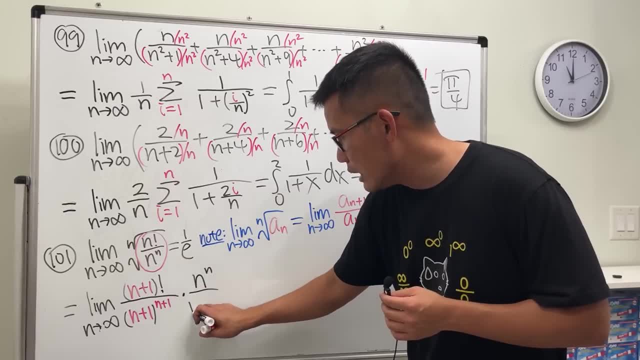 multiply by it's reciprocal, so i'm multiply by it's reciprocal, so i'm just going to put, just going to put, just going to put n to the n's power over n to the n's power over n to the n's power over n. factorial. 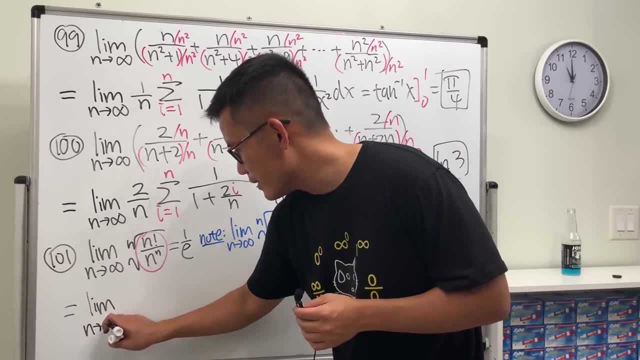 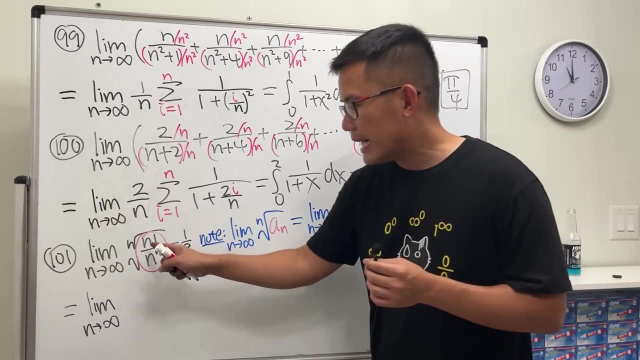 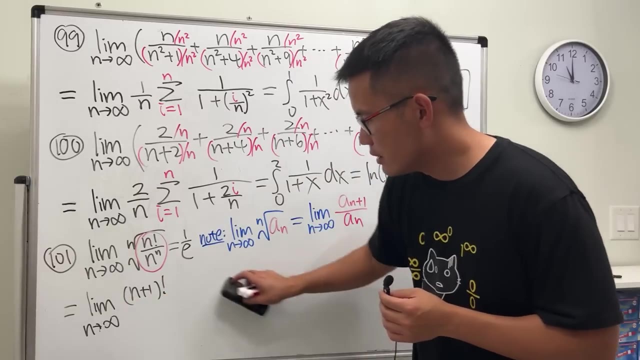 So this right here is the limit, as n goes to infinity. It's like whenever we have the nth root, just look at it inside and then just do a n plus one, meaning that we do n plus one and then we factorial that- sorry, n plus one. 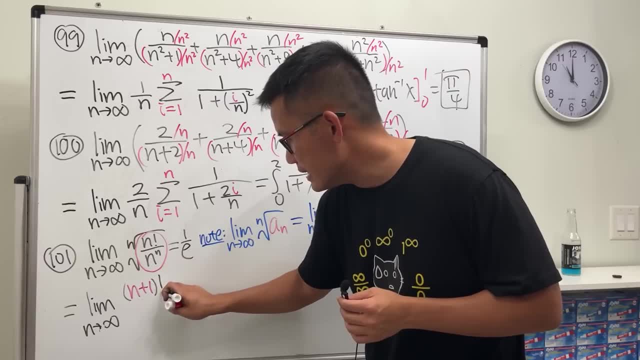 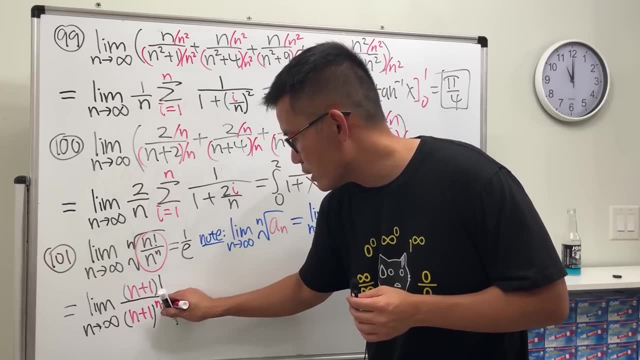 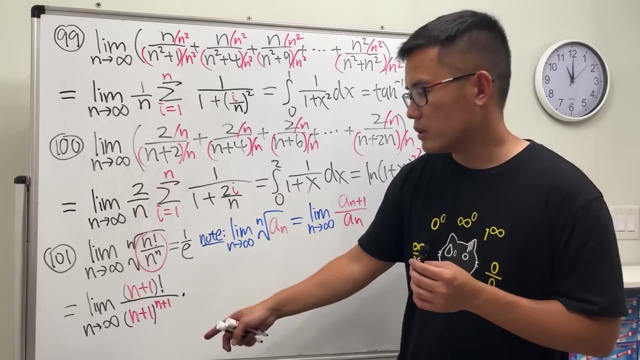 So n plus one factorial that, And then n plus one, raised to the n plus one. Okay, All right. All right, So n plus one power. And then we want to divide it by a n, which is the same as just multiply by it's reciprocal. 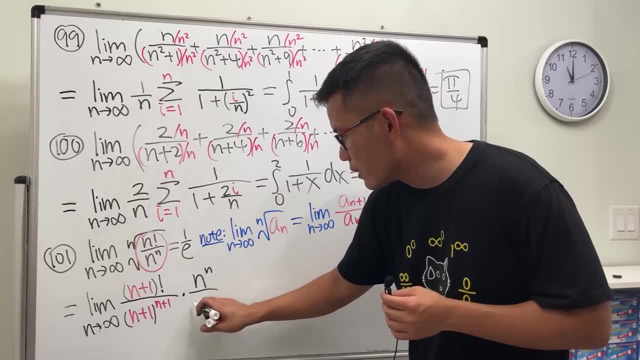 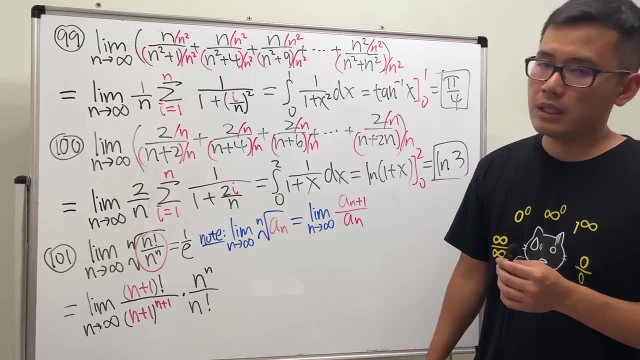 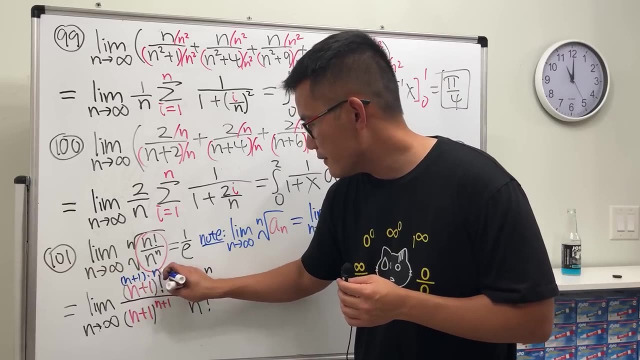 So I'm just going to put n to the nth power over n factorial. So if you have done some Calc 2 stuff, the ratio test or whatsoever, yeah, pretty much that. Now break this apart as n plus one times n factorial. 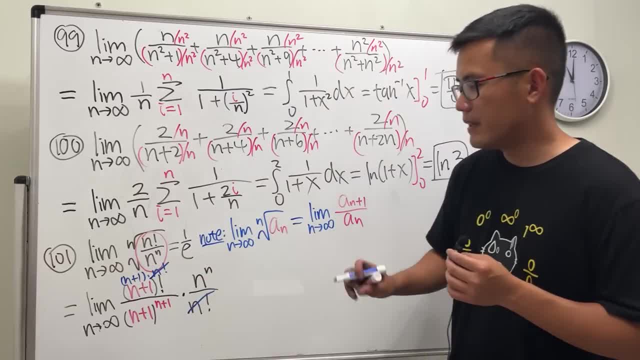 And you see that n factorial can solve Very nicely. What's this, though? We can also break it apart. Write this as n plus one to the nth power, first times n plus one to the first power, And then we see that it happens to be like n plus one, n plus one cancel, very nicely. 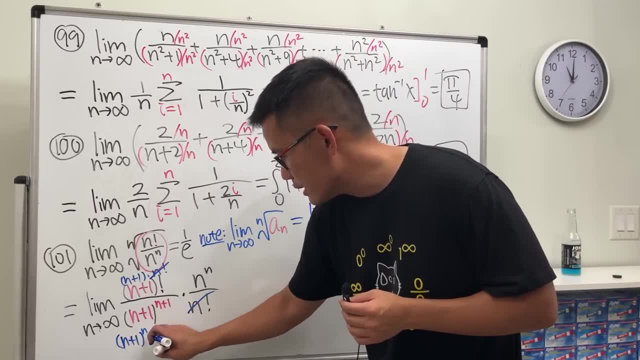 And this is so wonderful, because this has nth power, likewise that, So we can put them together as the ones n power, like this. So this is the limit, as n goes to infinity. Okay, Okay, Okay, Okay, Okay, Okay Okay. 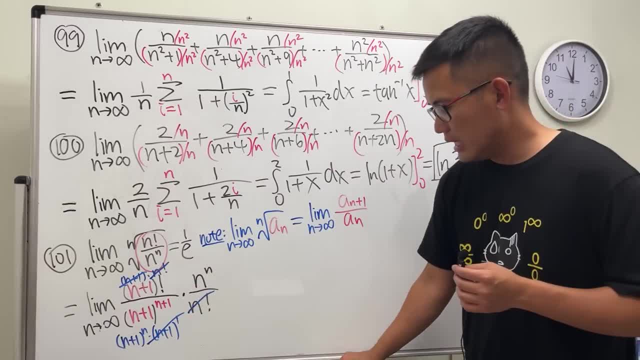 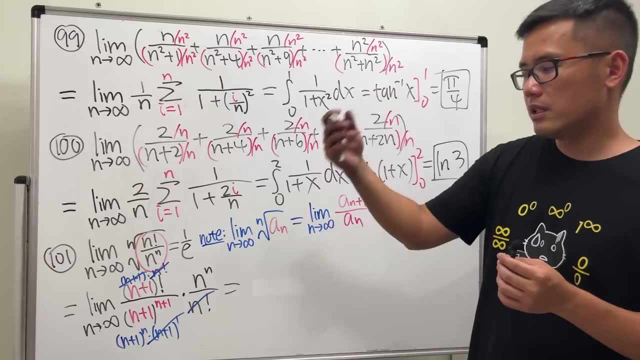 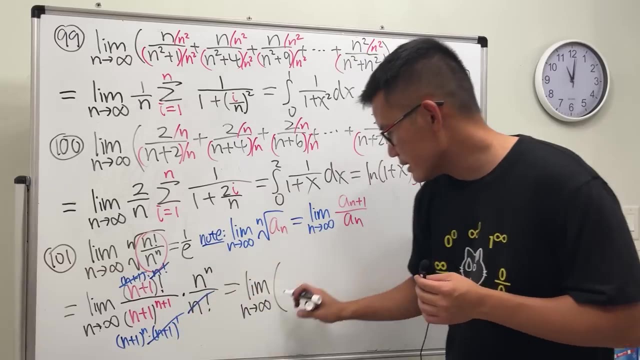 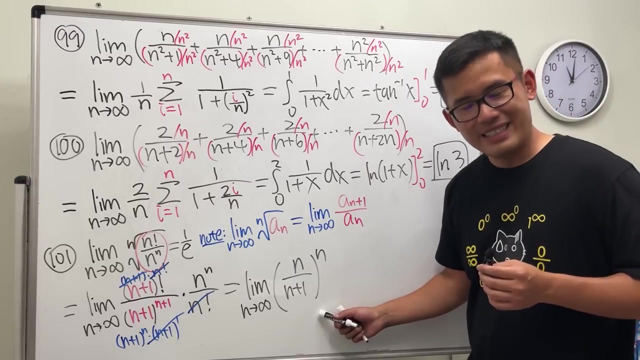 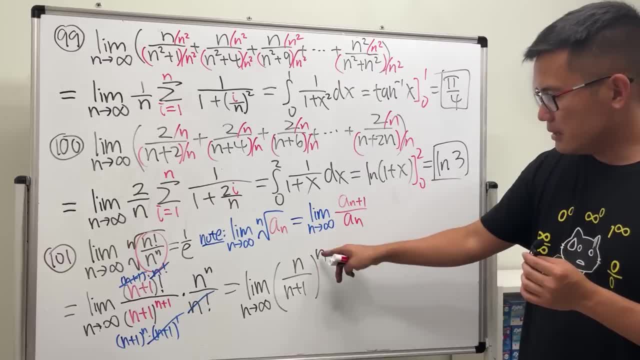 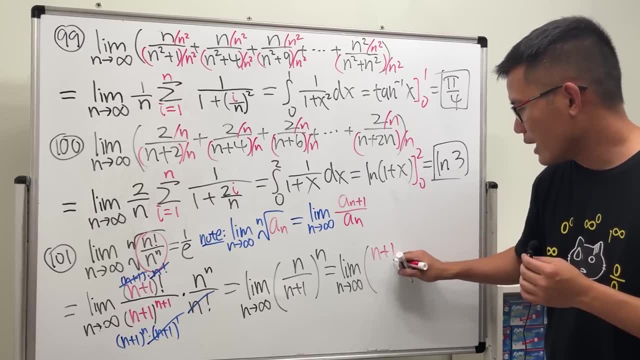 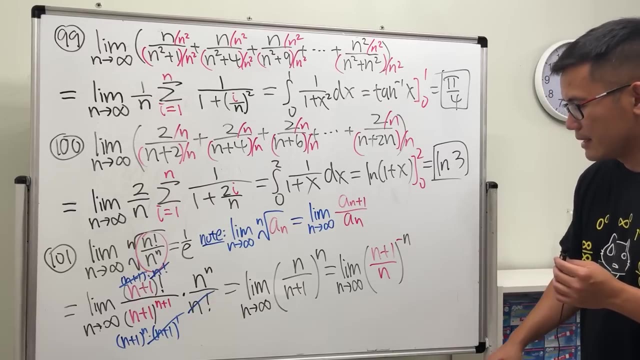 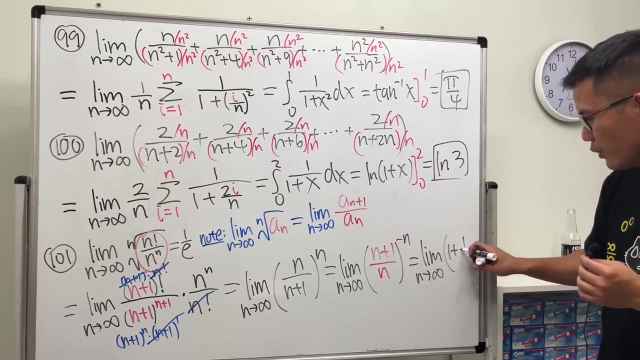 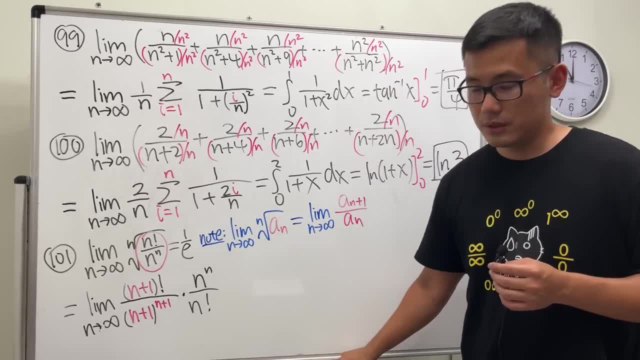 n factorial, n factorial. so if you have done some calc 2 stuff, so if you have done some calc 2 stuff, so if you have done some calc 2 stuff, the ratio test will whatsoever, the ratio test will whatsoever, the ratio test will whatsoever. yeah, pretty much that. 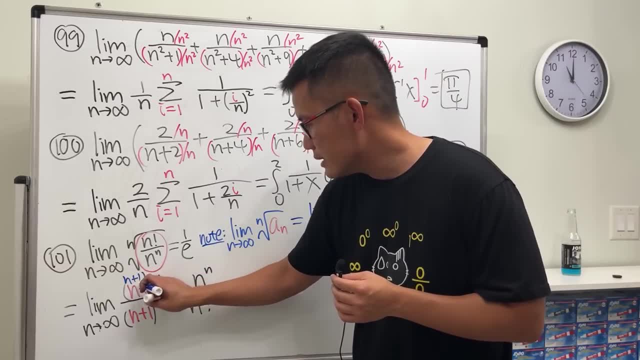 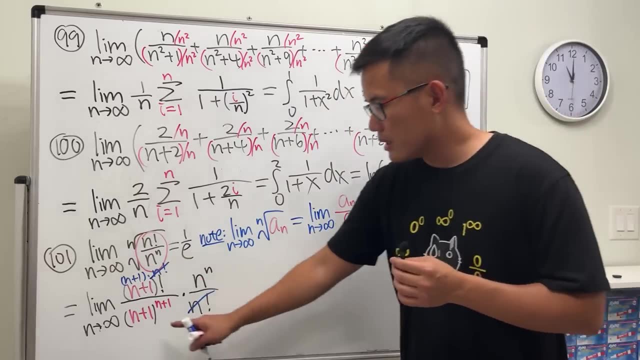 yeah, pretty much that. yeah, pretty much that. now break this apart as n plus one. now break this apart as n plus one. now break this apart as n plus one, times n factorial, and you see that times n factorial and you see that times n factorial and you see that n factorial can solve very nicely. 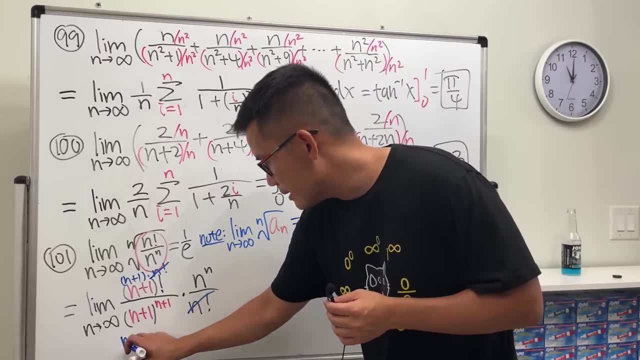 n factorial can solve very nicely. n factorial can solve very nicely. what's this, though? we can also break it. what's this, though? we can also break it. what's this, though? we can also break it apart apart, apart, right, this says n plus one to the nth. 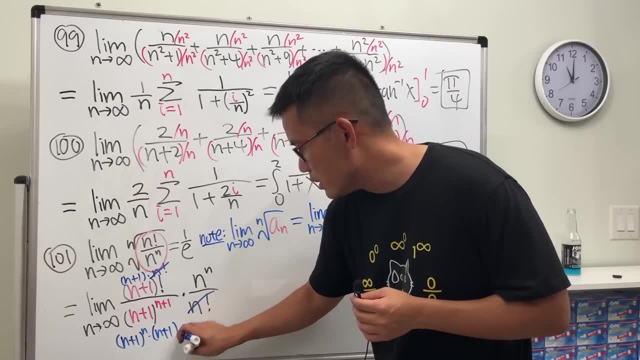 right. this says n plus one. to the nth right, this says n plus one to the nth power. first power, first power, first times n plus one times n plus one times n plus one to the first power. and then we see that to the first power, and then we see that: 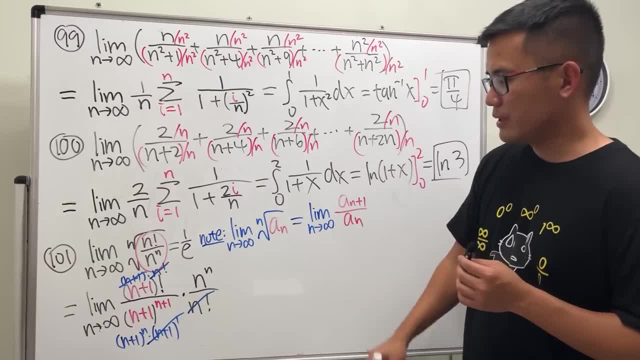 to the first power. and then we see that it happens to be like n plus one, n plus. it happens to be like n plus one, n plus. it happens to be like n plus one, n plus one. cancel, one, cancel, one, cancel. very nicely. and this is so wonderful. 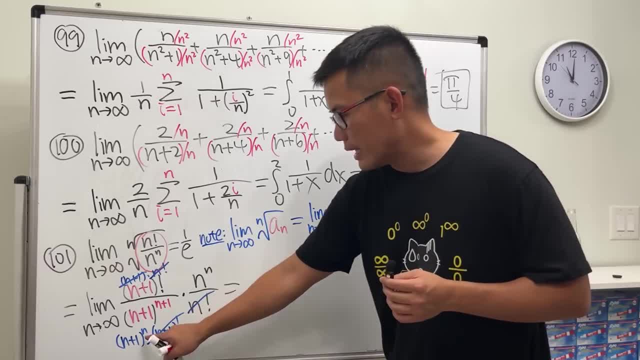 very nicely, and this is so wonderful very nicely. and this is so wonderful because, because, because this has the nth power, likewise that, so this has the nth power likewise that, so this has the nth power, likewise that, so we can put them together. we can put them together. 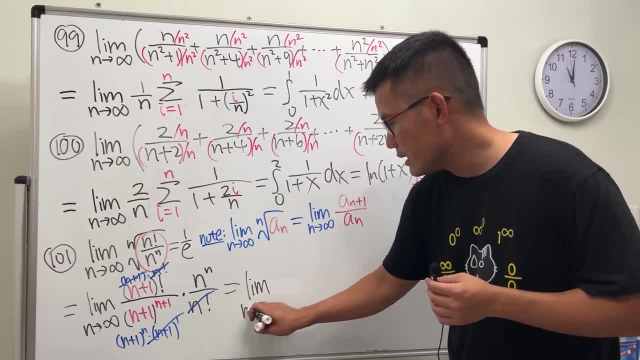 we can put them together as the ones and power like this. so this as the ones and power like this. so this as the ones and power like this. so this is the limit as n goes to infinity. is the limit as n goes to infinity is the limit as n goes to infinity and over that, so n over n plus one. 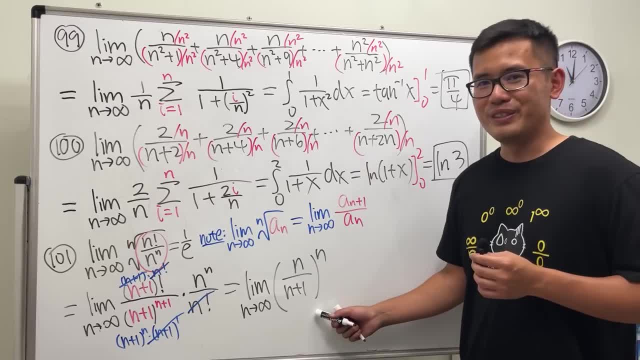 and over that, so n over n plus one and over that, so n over n plus one. power raised to the nth power. power raised to the nth power. power raised to the nth power. now. how do we do this now? how do we do this now? how do we do this? we have done something like this, right. 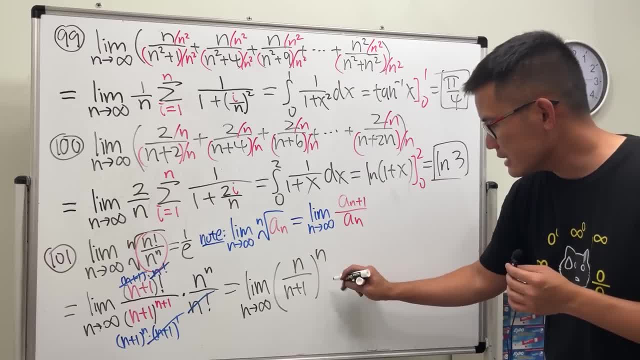 we have done something like this, right. we have done something like this right. yes, the secret weapon. yes, the secret weapon. yes, the secret weapon. flip this. negate that here. this is the flip this. negate that here. this is the flip this. negate that here. this is the limit, as n goes to infinity. 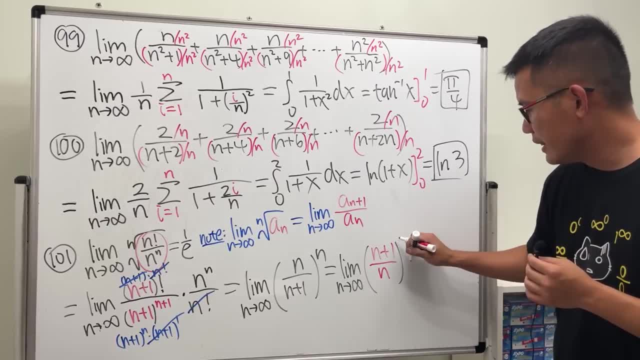 limit as n goes to infinity, limit as n goes to infinity, n plus 1 over n raised to the n plus 1 over n raised to the n plus 1 over n raised to the negative nth power. and you know it. this, right here is just. 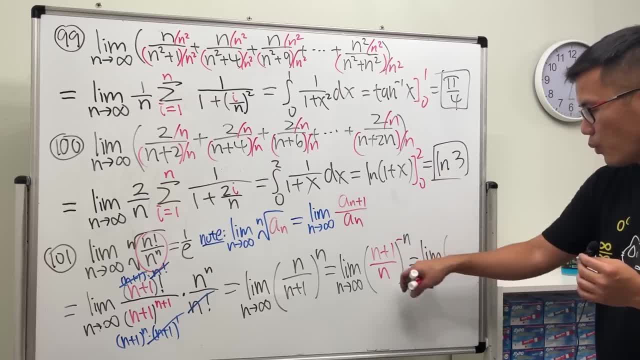 and you know it, this right here is just, and you know it, this right here is just the limit, the limit, the limit as n goes to infinity 1, as n goes to infinity 1, as n goes to infinity 1 plus 1 over n raised to the 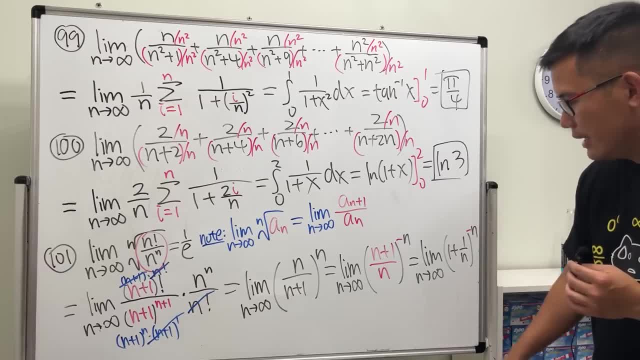 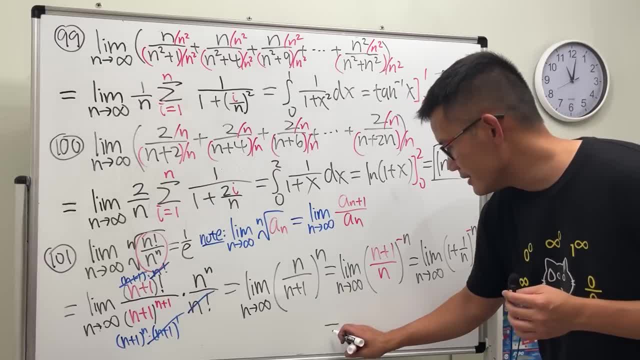 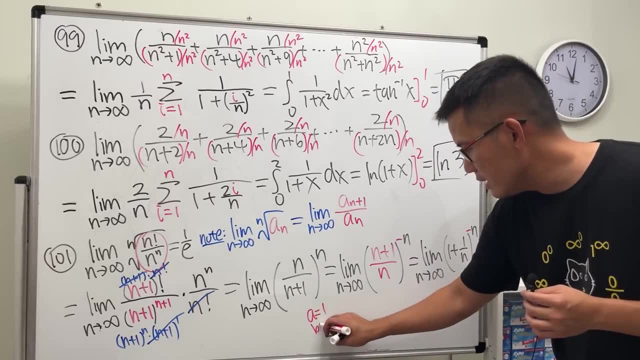 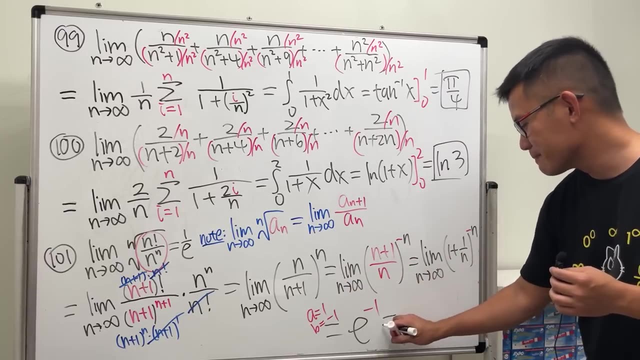 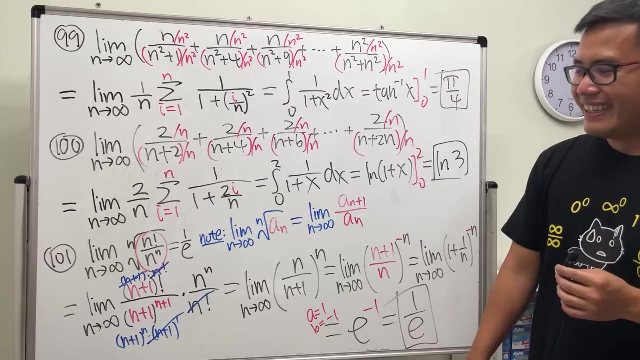 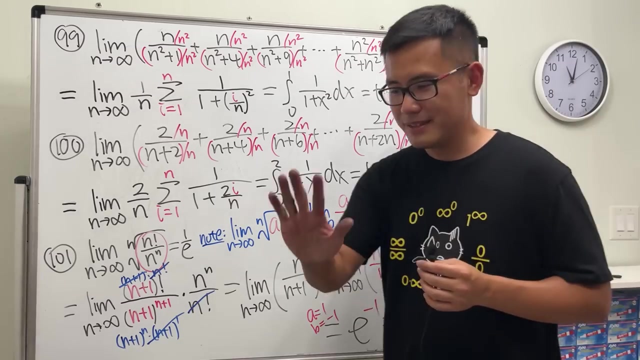 and you know it, ladies and gentlemen: a is 1, b is equal to negative 1, so, all in all, the answer is e to the 1 times negative 1, which is negative 1. this is how dirty my hand is. yeah, because this thing is so dirty. uh, i should wash it. 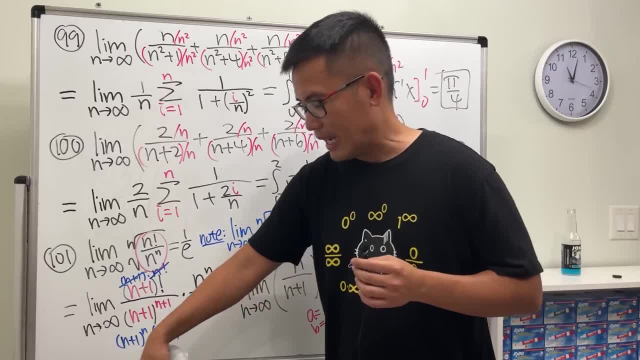 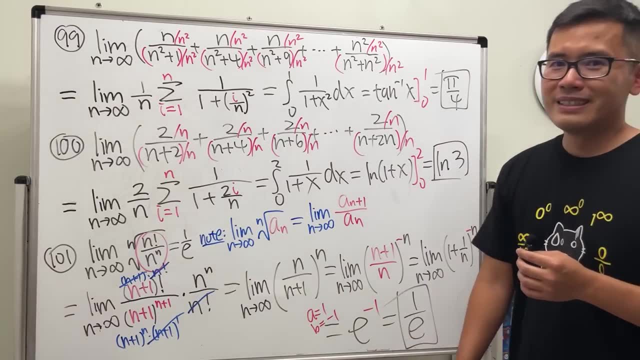 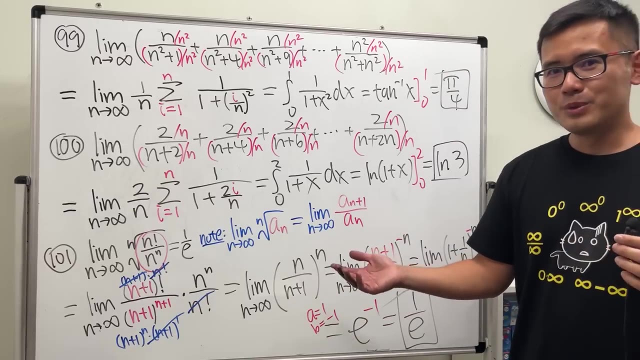 yeah, i do wash it occasionally, like every other week or so. yeah, i have a couple of those. but anyway, though, 101 limits you, hopefully this video can help you with your calculus 1, calculus 2 class. if you're my students, hopefully you're watching it. 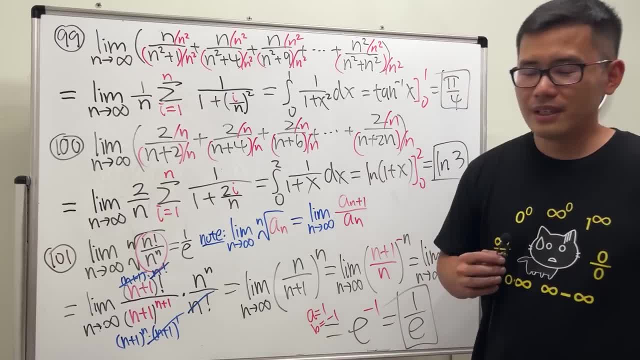 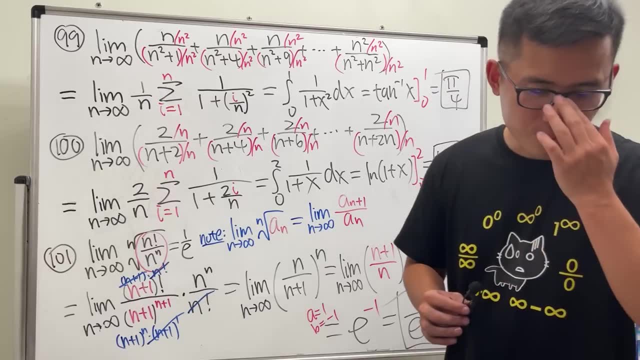 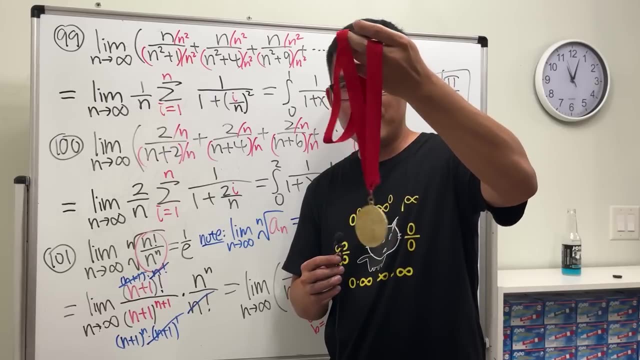 maybe i'll pick some questions from here to be to put on a test. yeah, and you know it. i told you guys i run marathons, so i'll show you guys. yes, this is the marathon medal that i have. yeah, the very first one definitely means the. 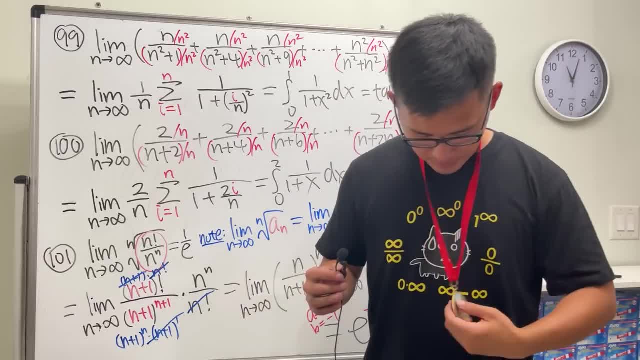 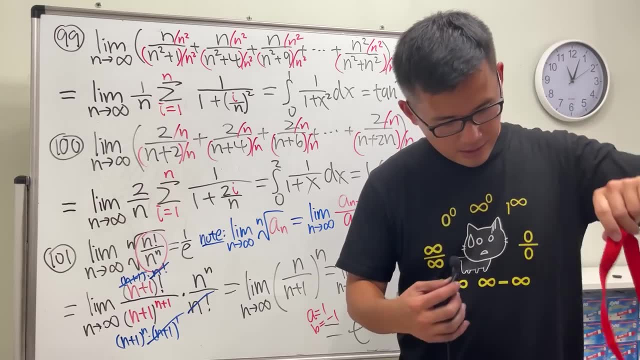 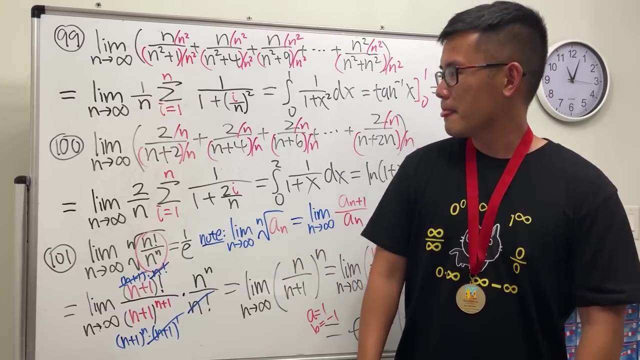 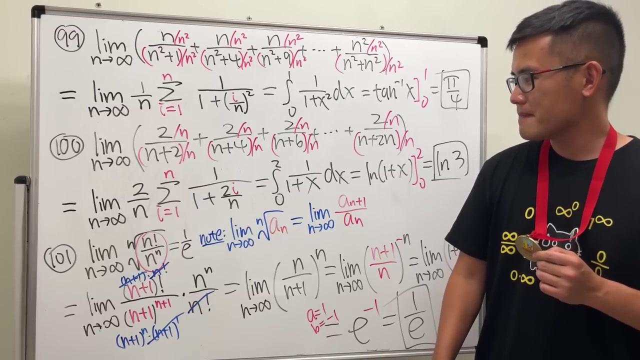 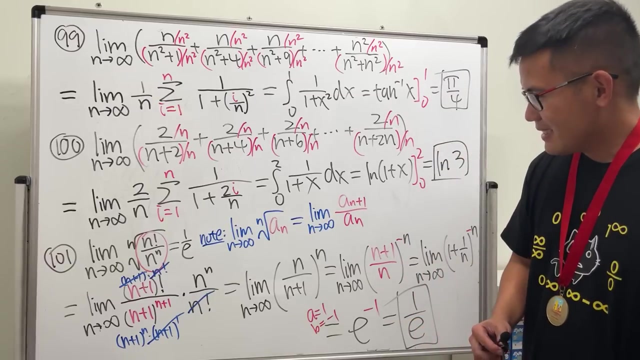 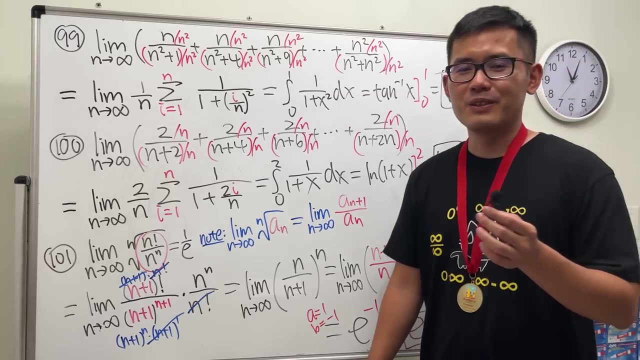 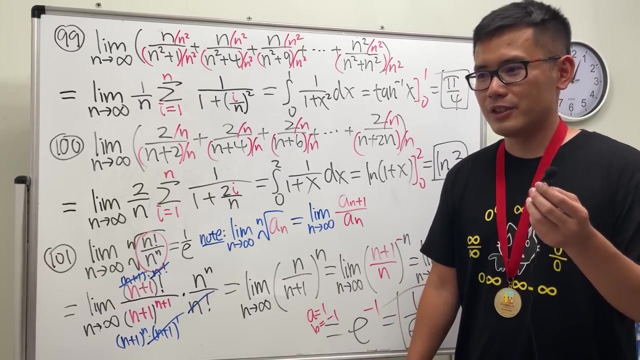 most to me. ah, let me. oh. so finally, you have some limits. i- i don't know what else to say. thank you guys so much. thank you for all my subscribers, all my viewers and all the sponsors, all my patreons and all my channel members, everybody. 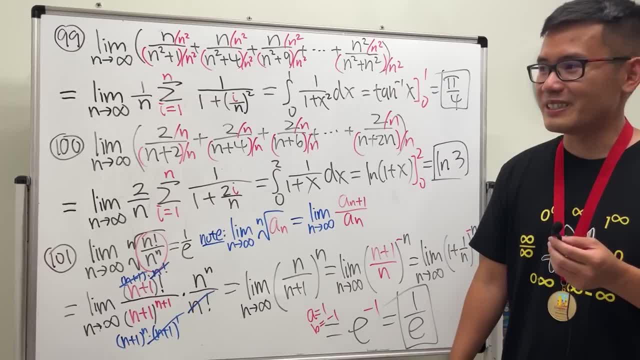 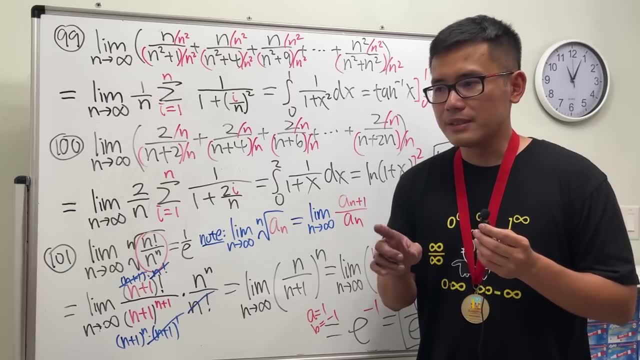 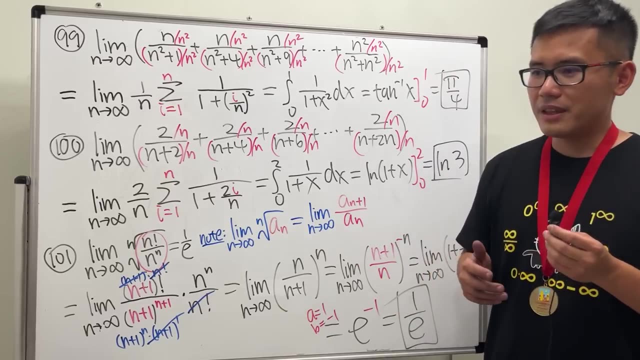 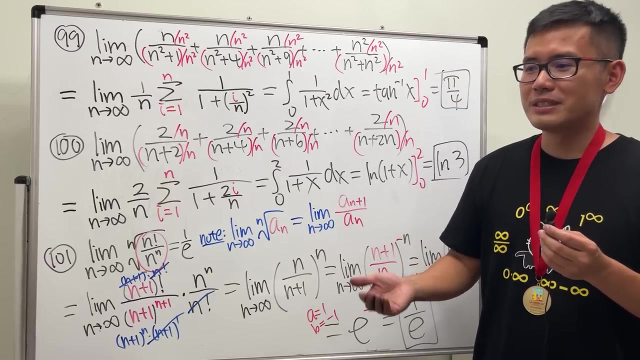 almost one million subscribers. can you just believe that insane fun fact? i remember i reached- I reached 10,000 subscribers on October 20th 2016. so you will be kind of interesting or funny that I reach exactly 100, exactly 1 million subscribers on the same day, but six years later now. that's kind of cool. I 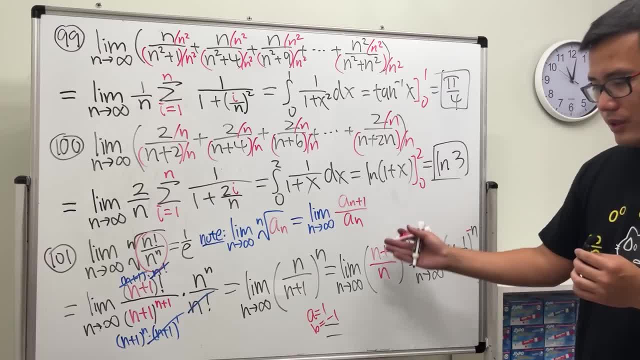 is is 1: 1. 1 b is equal to negative 1. so all in all, b is equal to negative 1. so all in all, b is equal to negative 1. so all in all, the answer is e to the. the answer is e to the. 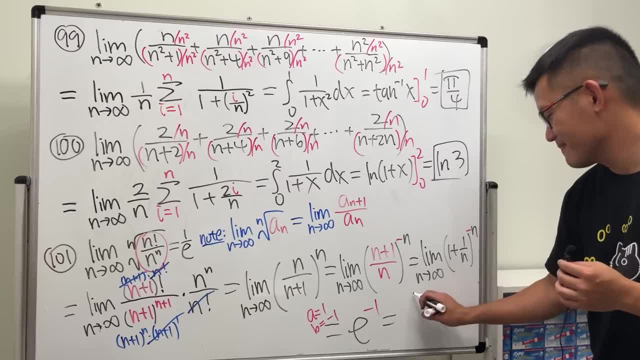 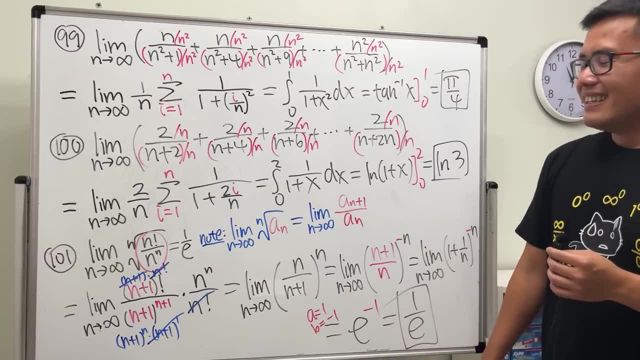 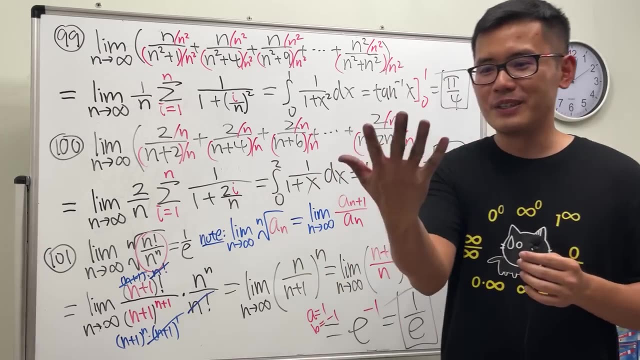 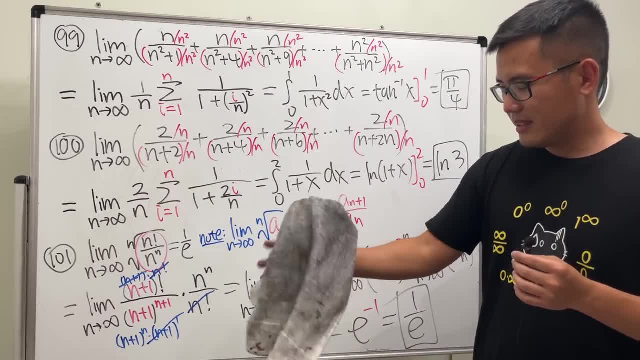 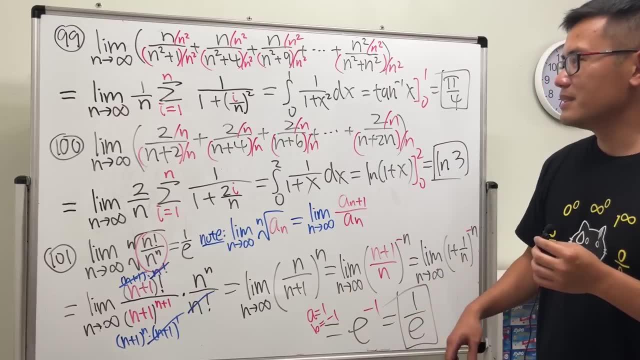 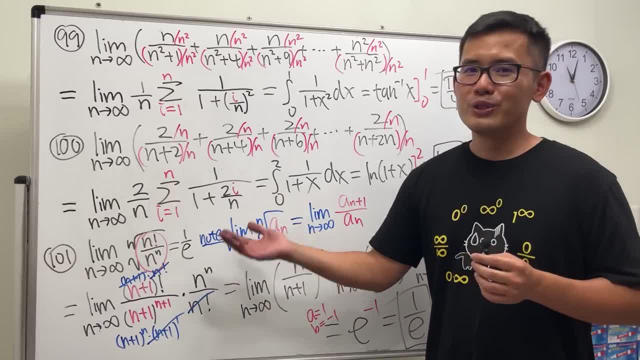 every other week or so. yeah, i have a every other week or so. yeah, i have a couple of those, couple of those, couple of those, by the way, though 101 limits, by the way though 101 limits, by the way though 101 limits, hopefully, this video. 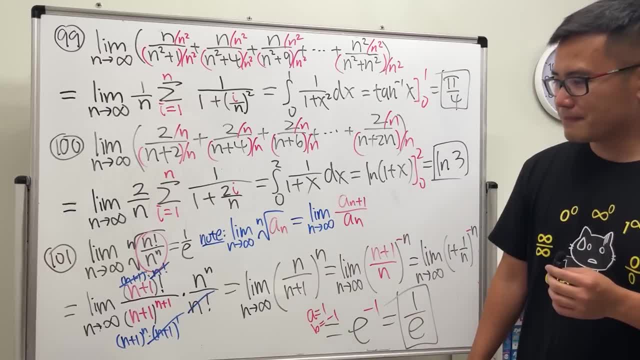 hopefully this video, hopefully this video. i can help you with your calculus one. i can help you with your calculus one. i can help you with your calculus one, calculus two class, calculus two class. calculus two class. if you're my students, hopefully you're. if you're my students, hopefully you're. 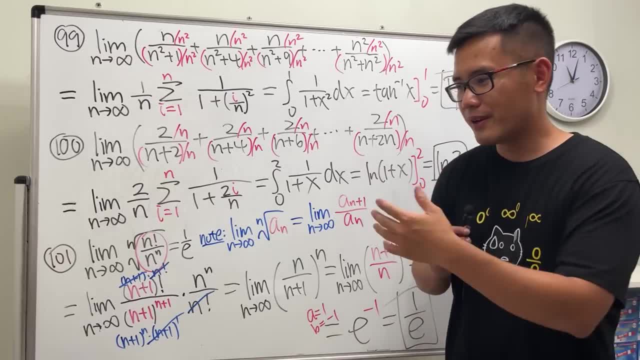 if you're my students, hopefully you're watching it, watching it, watching it, uh. maybe i'll pick some questions from uh. maybe i'll pick some questions from uh. maybe i'll pick some questions from here to be here, to be here to be to put on a test. 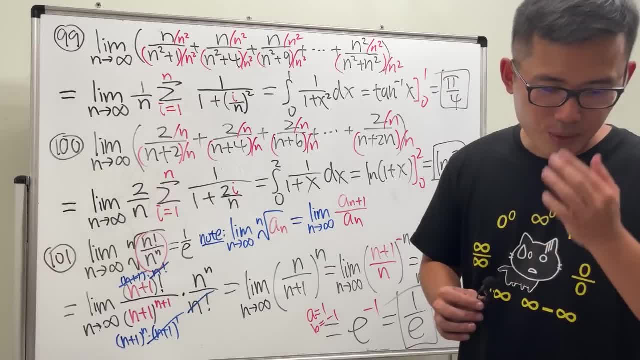 to put on a test. to put on a test, yeah, yeah, yeah, and you know it. i told you guys i run and you know it. i told you guys i run and you know it. i told you guys i run marathons, so i'll show you guys. 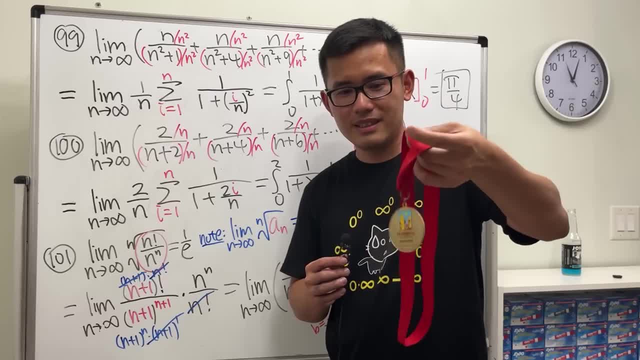 marathons. so i'll show you guys marathons. so i'll show you guys: yes, this is the marathon metal that i, yes, this is the marathon metal that i, yes, this is the marathon metal that i have have have. yeah, the very first one. yeah, the very first one. 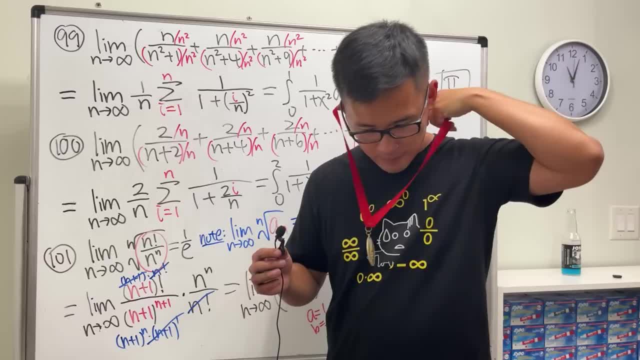 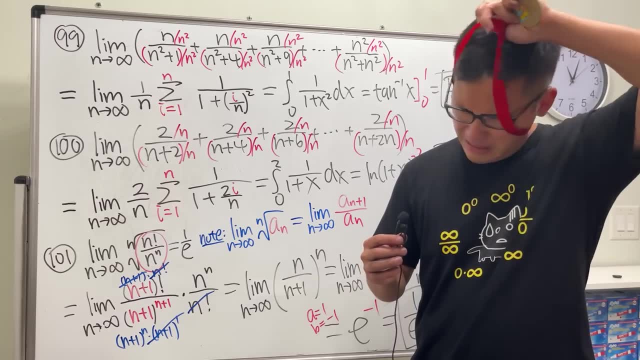 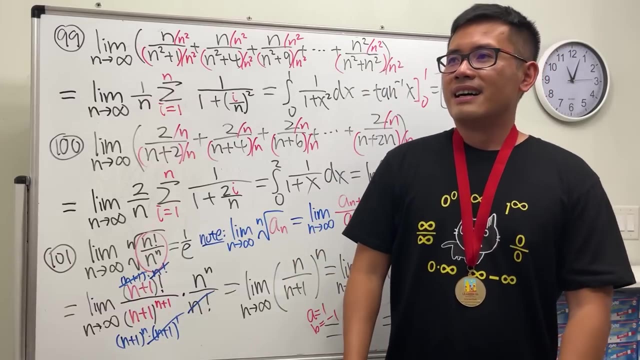 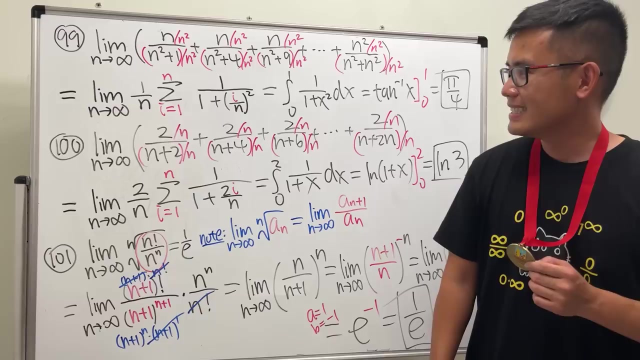 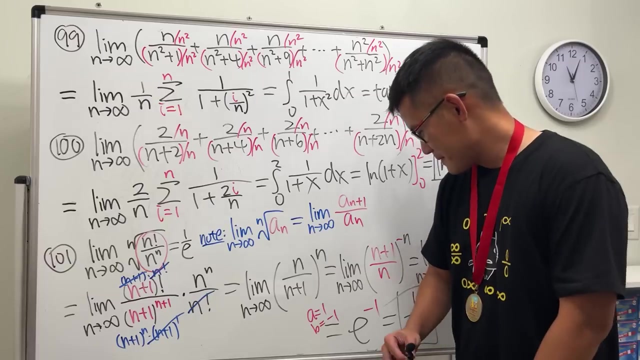 yeah, the very first one definitely means the most to me, definitely means the most to me, definitely means the most to me. now put it up, now put it up, now put it up. oh so, finally you have some limits. so finally you have some limits. so finally you have some limits. i- i don't know what else to say- thank. i- i don't know what else to say. thank i. i don't know what else to say. thank you guys so much. thank you for all my you guys so much. thank you for all my you guys so much. thank you for all my subscribers, all my viewers.